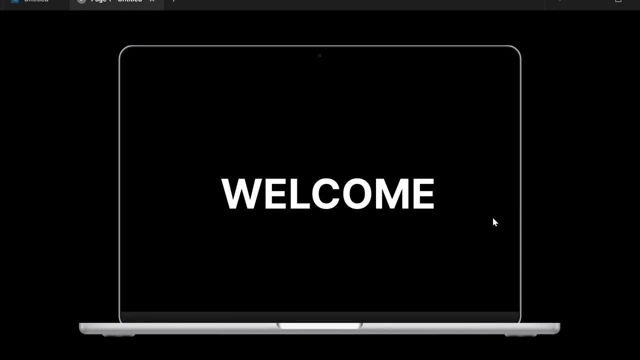 challenges I give you if you do all of the projects which I'm going to be doing throughout this course. So by the end of this course, you will be able to create your own markups by using HTML and CSS. So enough talking. Now let's just see what we are going to be learning throughout. 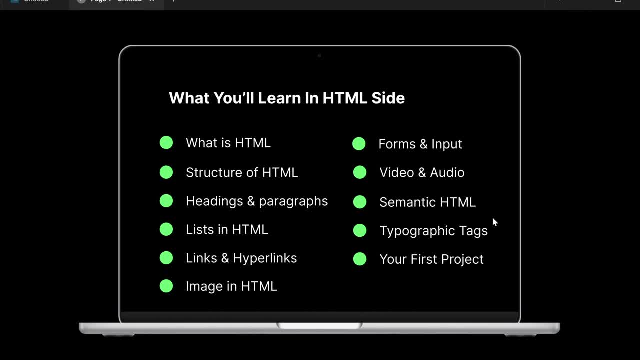 this course. So, first of all, we are going to be starting our journey by learning about HTML. So, like we are going to be learning what HTML is and structure of HTML, and all of these topics which you can see on the screen right now, then we are going to be learning. 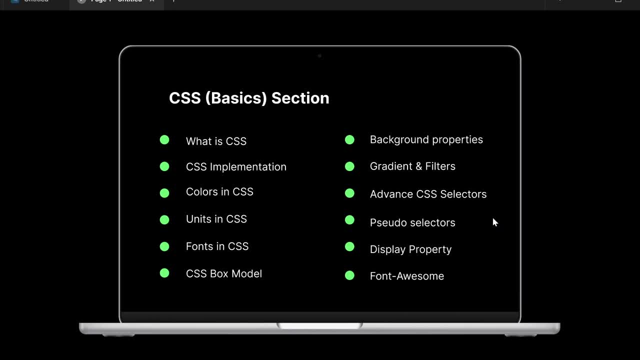 about the basics of CSS, like what a CSS is, CSS syntax, implementation, colors, units, fonts and etc. etc. After that, we are going to be jumping into something called a flexbox And we are going to be learning crazy amount of stuff about flexbox. Okay, so after that we are going 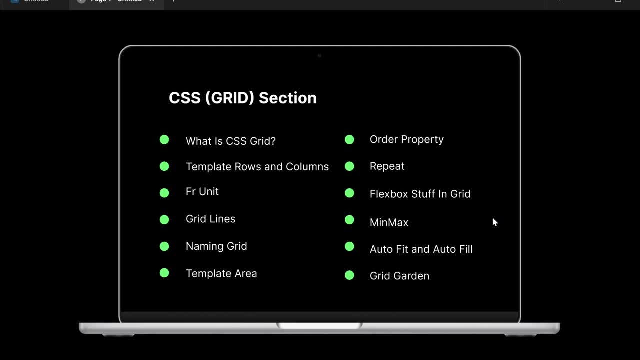 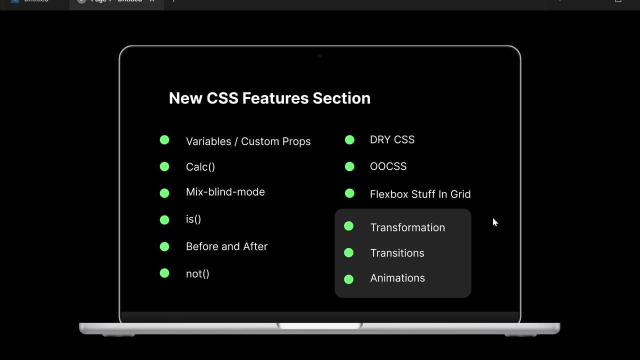 to be learning about what a CSS grid is and then like how all of that grid works in CSS, And then we are going to be learning about the basics of CSS. So after that we are going to be learning about new feature in CSS, like what is a variable called mixed blending mode is before and after. 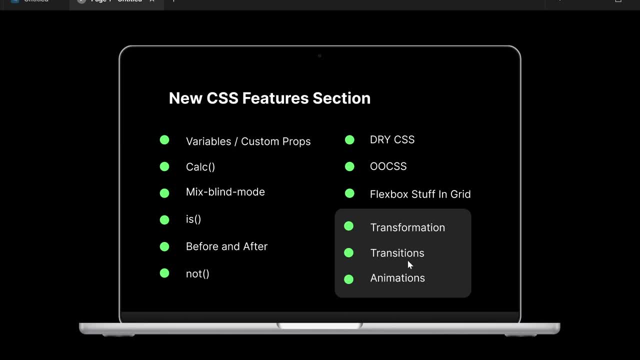 and that stuff, And I don't want to make another slide, So I put this old stuff as well. So we are going to be also learning about transformation, transition and animation by the end of this course. After that we are going to be building or awesome, awesome projects. Okay, so suit for. 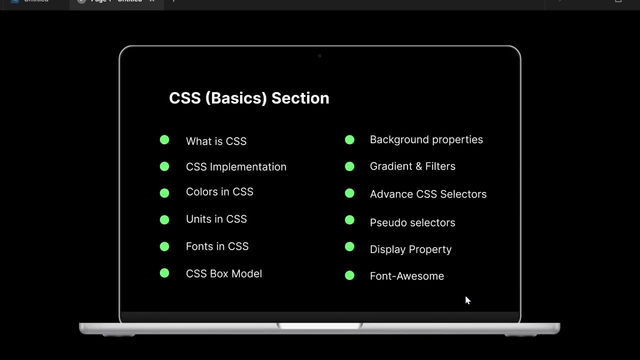 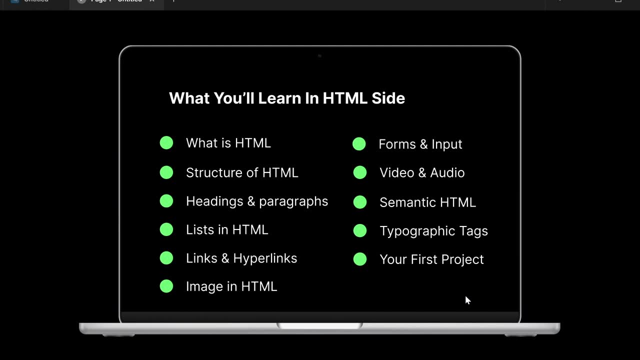 yourself, if you know all of this stuff. So you can just pick, like wherever you want to start from this course. If you're completely beginner, like if you don't have any idea like what HTML and CSS even means, So you should start from the beginning And I want to welcome you all. So the next thing which you have to do is that we 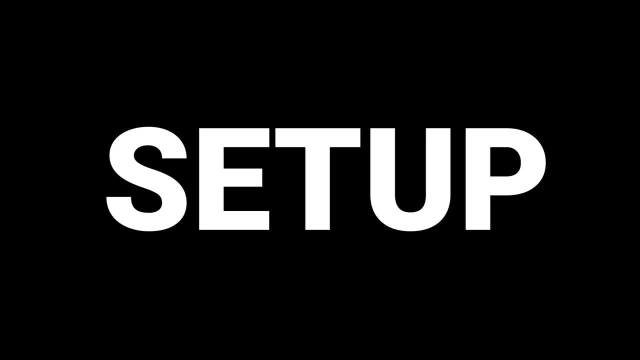 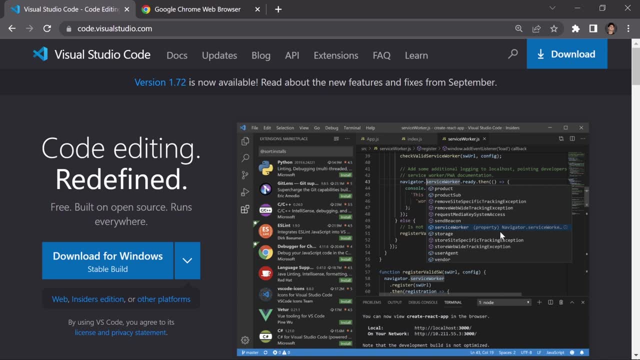 have to make a setup for our coding journey. All right guys. so before getting into the actual content of this course, first of all we have to make setup for our coding journey so that we can write our code somewhere and we can test the result of our coding somewhere. So for this, 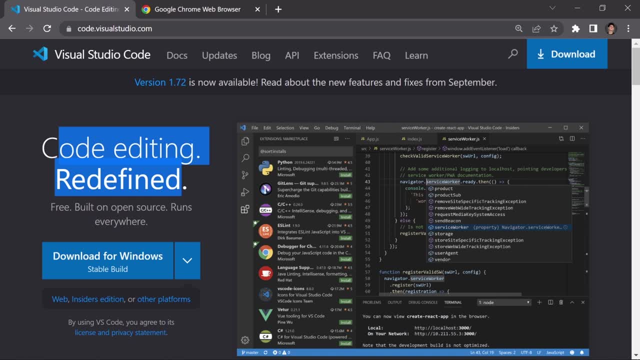 course, we are going to be using something called a virtual story coder And which allows us to write our code And you are totally free to choose whichever kind of quarter you like. Like you can use sublime text, you can use Adam and stuff like that. There are. 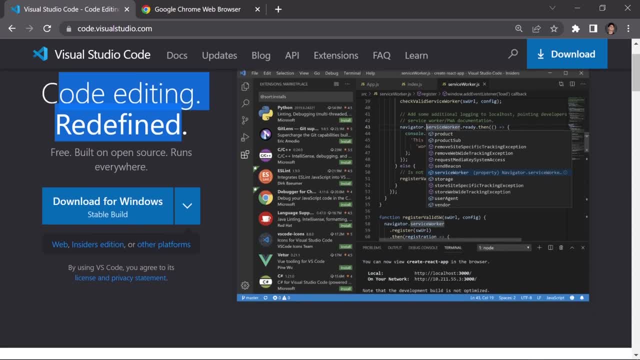 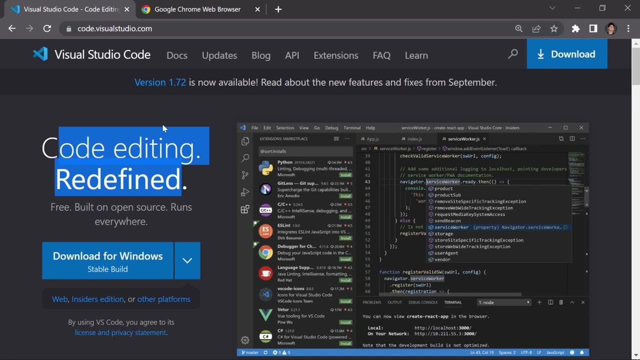 a lot of quarters out there. If you want to choose some others, So you can also choose that, But my recommendation will be to use a visual story coder, And you are totally free to choose whichever you like. Anyways, so if you want to download and install a visual story coder in your machine, 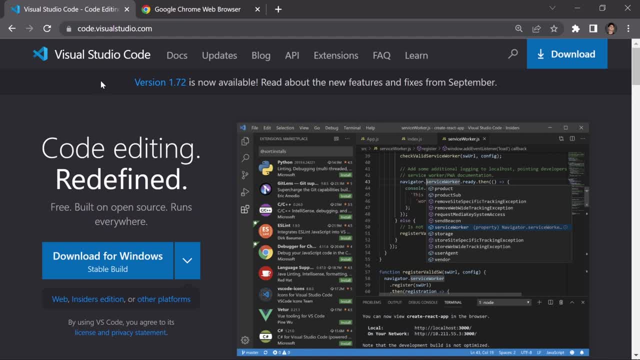 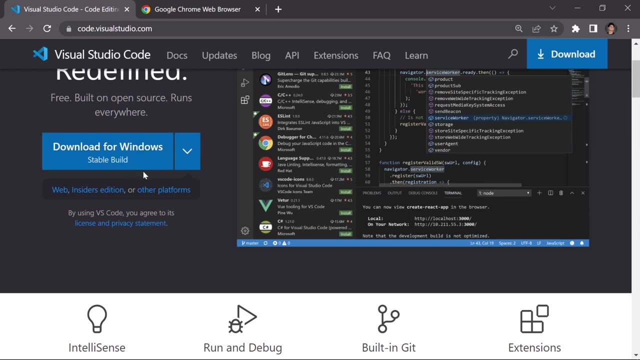 so I'm going to give you this link So, like you can just click on there, it will bring you to this page right here, okay, And it will by default detect your operating system. So I'm using a Windows And I don't know if you're using, like Mac OS or Linux or whatever kind of operating. 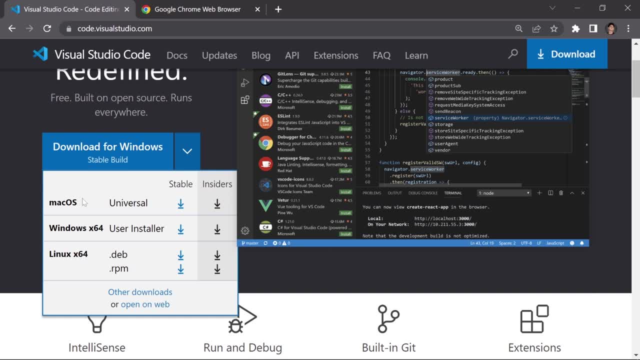 system you're using, But you can install it for your own operating system, Like here. you can see, we have option for Mac OS users, we have for Windows user and we also have an option for a Linux user. Okay, so I want you to just click on this button, or you can just 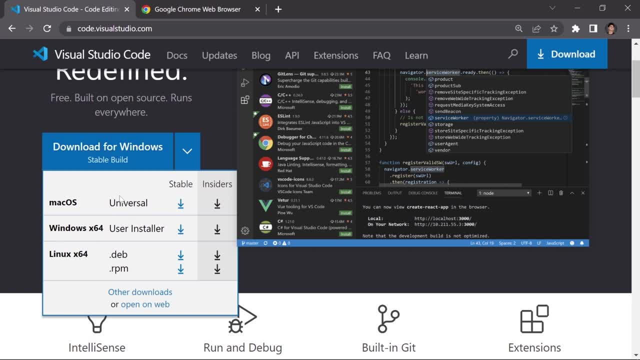 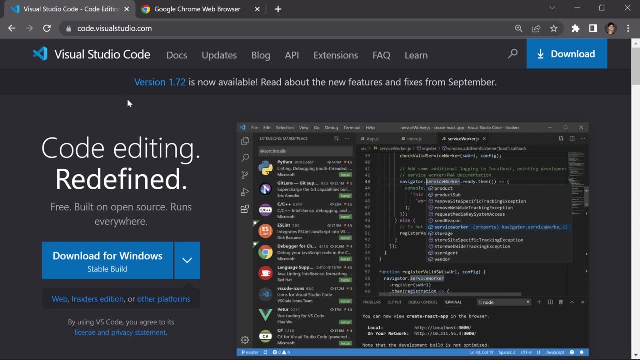 download it for your own specific operating system. So this is how you do that: And then hit next, next, next, and just install it in your operating system. It's not that much hard. And now the next thing I want you to download and install in your machine is something called a web browser. 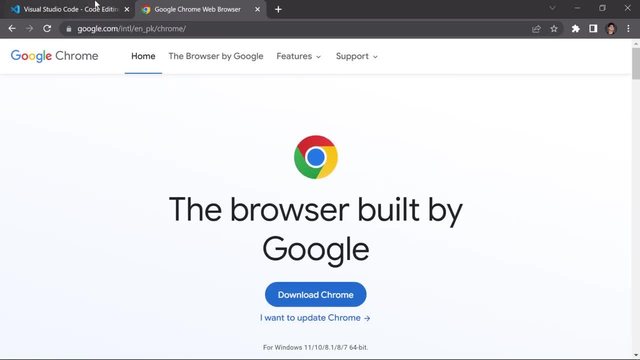 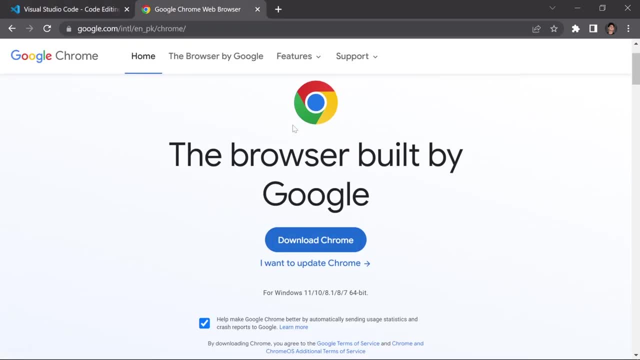 in which you are going to be testing the result of our coding. So in Visual Story coder, we are going to be writing our code like here- you can see that- and in web browser, and you can choose whichever kind of web browser you like, but not an Internet Explorer. Okay, you can choose whichever. 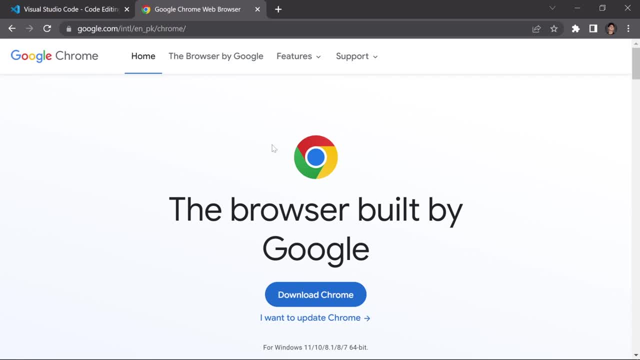 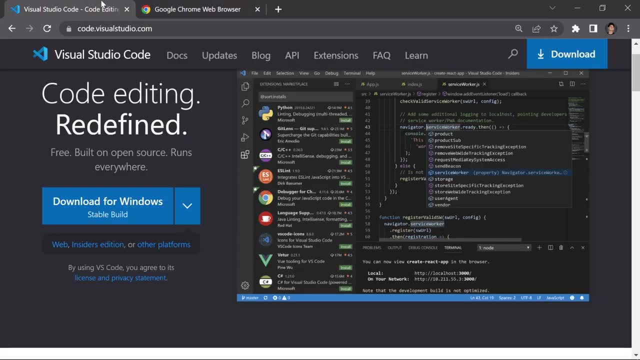 kind of web browser you like, like Chrome or Safari, I don't know, like whichever kind of browser you like, but not Internet Explorer. Okay, so this is it for the setup. I want you to just go to these links and download and install it into your machine, And then you're going to be ready. 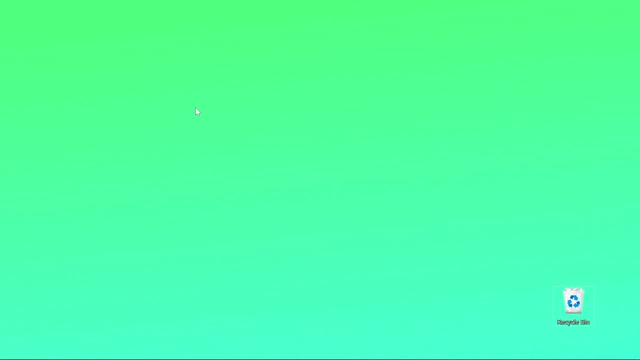 to go. So now, the next thing which you have to do is that you have to create a folder somewhere. So in their folder we are going to be writing our code. Okay, so in my case, I'm going to just create my folder inside my desktop And you can create it anywhere you like. And now I'm gonna give a name. 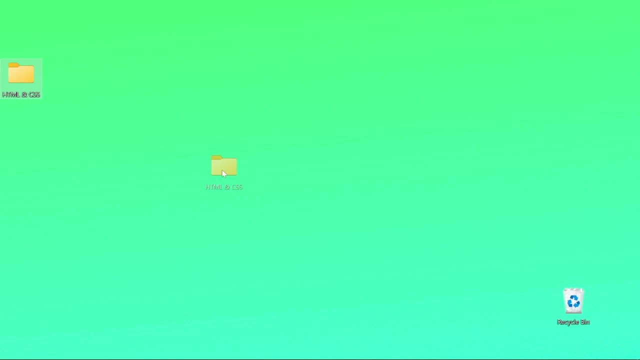 of like HTML and CSS And you can give them any name you like. And now what do I have to do? I'm going to just open my terminal, like oh you know what? I'm going to just open my Visual Story coder, right? 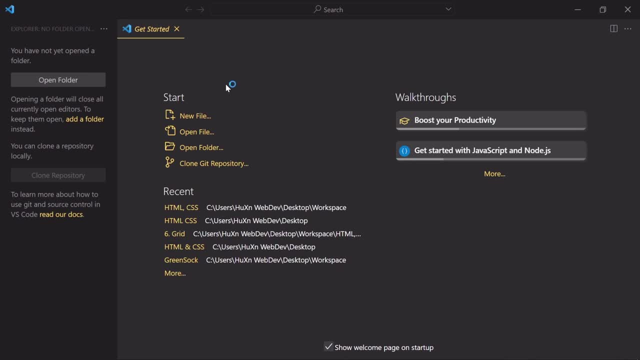 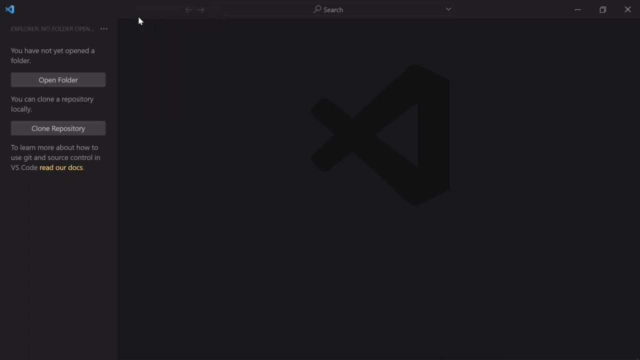 here. So, and now here you can see, I launched my Visual Story coder right here, And chances are your coder will not look the same like mine. your coder will look like this, like the menu bar, will look like this, And chances are you won't have this search bar in there. you don't have to worry. 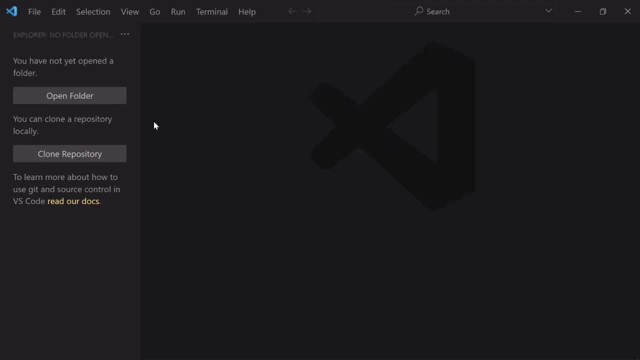 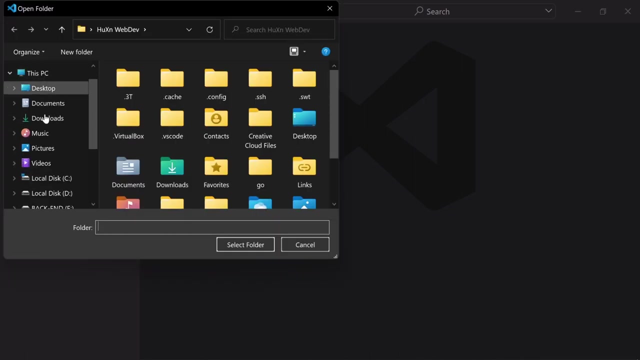 about all of this stuff for now. So now the thing I want you to mention is that if you want to open your folder in a Visual Story coder, so you can either just click on this open folder button And then you can choose like: where is your folder located In my? 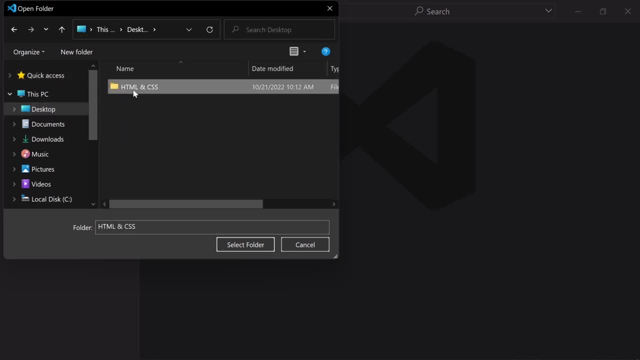 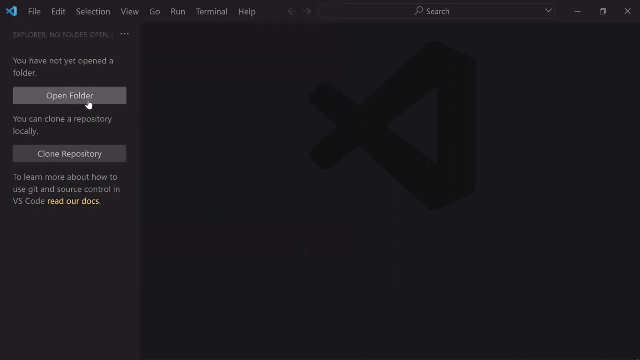 case it's on the desktop. So I'm going to just click on a desktop And then I can choose my folder from there And then I can just click on this select folder. In your case, if you don't have like this open folder button, chances are you will have this live open folder button. But 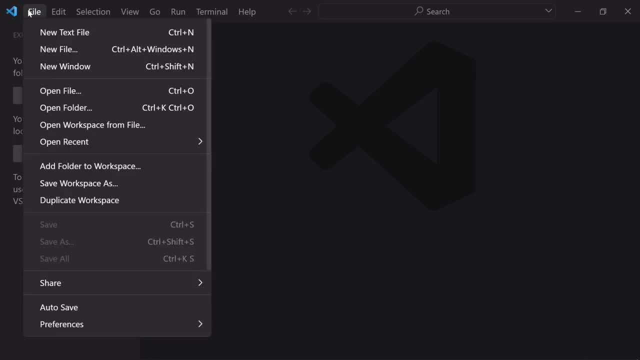 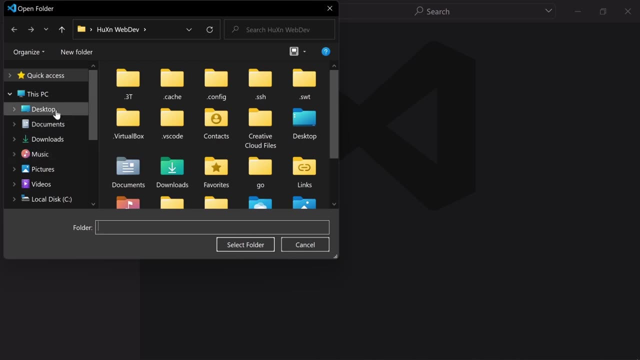 if this is not available or you cannot see that, so you can just click on this file button and then click on this open folder. So it will also give you that same pop up box right here. So you can then just click on this desktop. 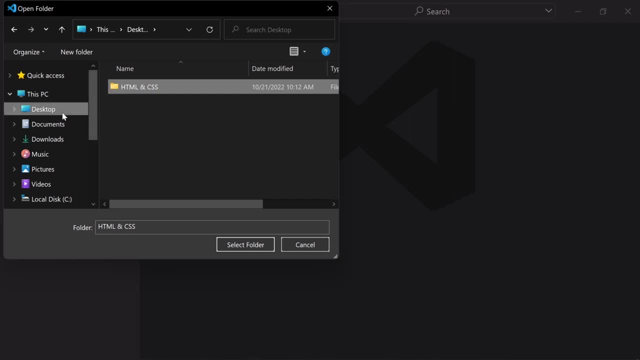 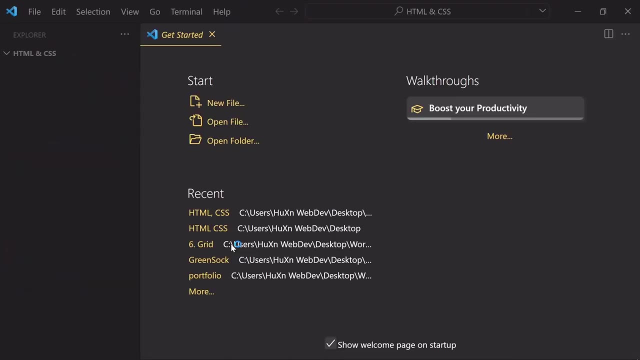 and then click on your folder. Okay, so in my case it's on like desktop and then we have HTML and CSS, And now I'm going to just click on this select folder for now. So it will now open this folder in my Visual Story coder. So here you can see. our folder is totally empty, So we don't. 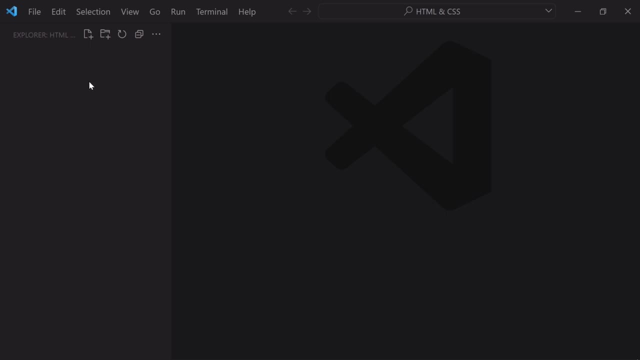 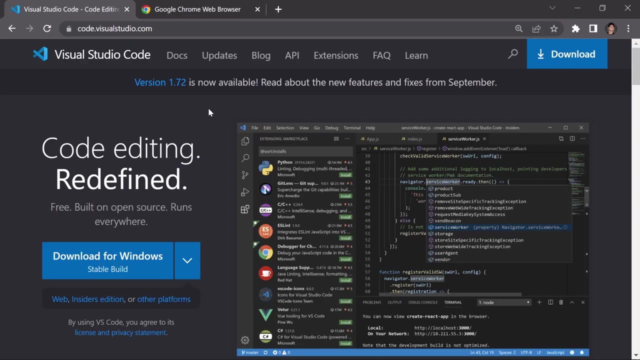 have any files and then like any content whatsoever right here. So now, here you can see this totally empty. So now, if you want to work with the HTML, first of all let's just learn about like what in the world is HTML, and then we are going to writing or coding. So in this course, 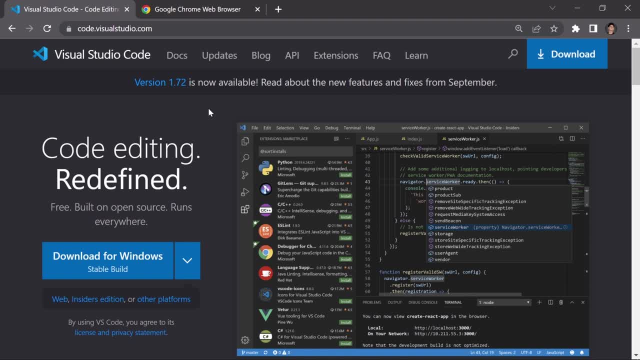 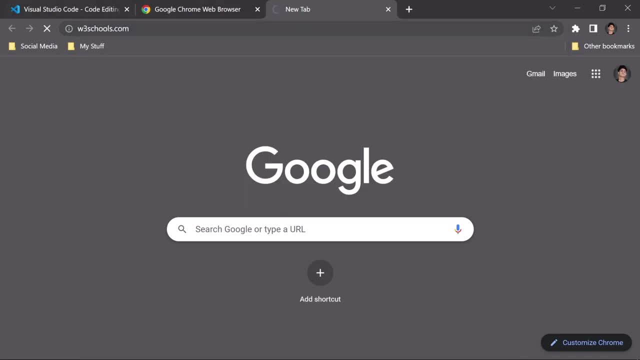 you'll have two friends, or maybe more than two friends, But in my opinion these two will be your best friend. The first one will be MDN And the second one will be w three school. Okay, so you just have to type like w three school, comm, And then it will bring you to this web. 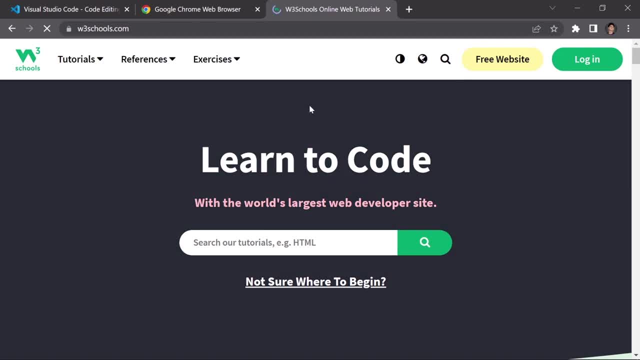 page right here, And I guess by default your web page will look like this, like a white one. then you can just hover your mouse over to this kind of uh, um, i can't even call this um- you just have to roll your mouse over to this icon and then click on this dark mode right here. so it will now. 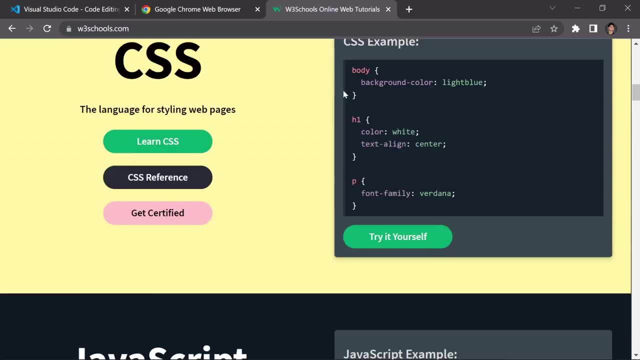 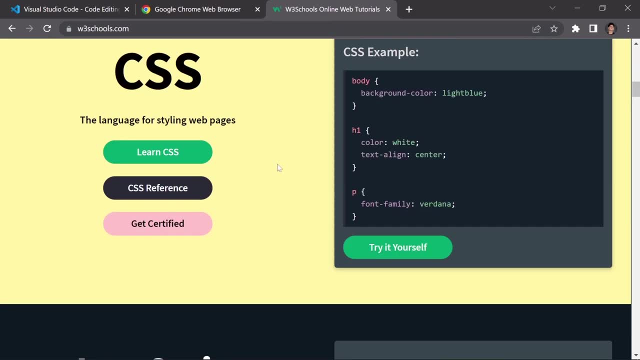 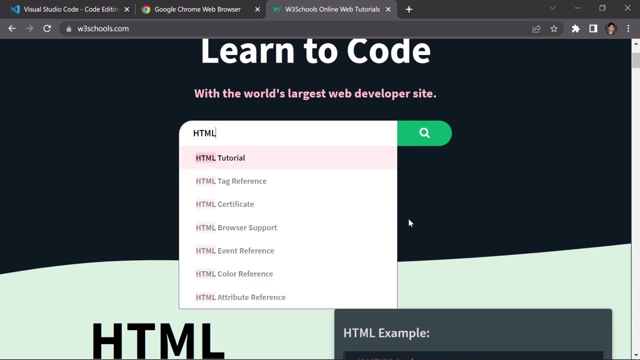 provide you with a dark mode, and here you can learn crazy stuff about html. this is javascript, sql, php and a lot of crazy technologies like that, but you don't have to go to that much detail. so now let's suppose if you want to search for html, so i'm going to just write html, and now i'm going. 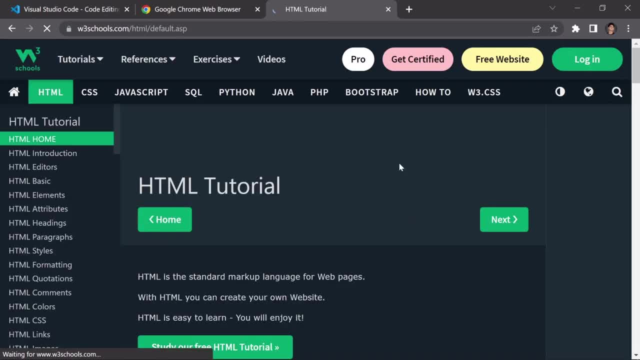 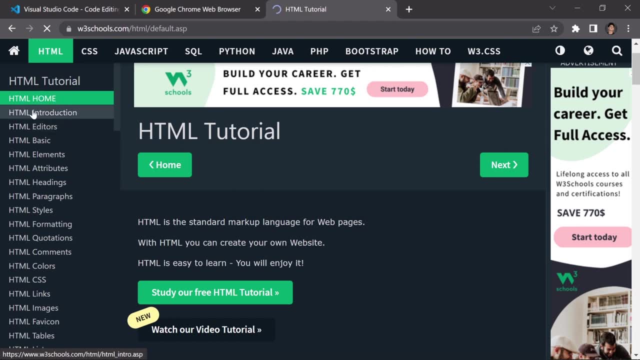 to hit enter right here, or you can also click on that search. and now, here you can see, tom log uses these definition. so we are not going to be clicking on this html home, we are going to be clicking on html introduction. so i'm going to just click on that. and now, here you can see, for now you. 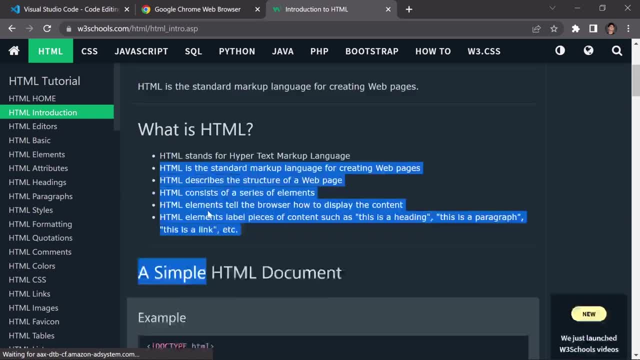 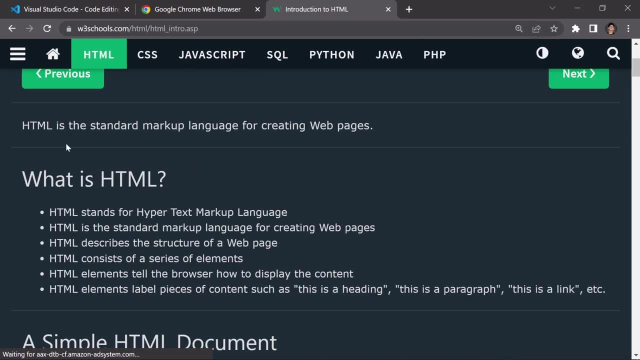 don't have to worry about all of these crazy syntax and stuff for now, but i want you to just notice two things. so i'm going to just zoom in a bit so that you guys can see everything a bit clear. so first of all, i want you to know that what is html? html is just a standard markup language for 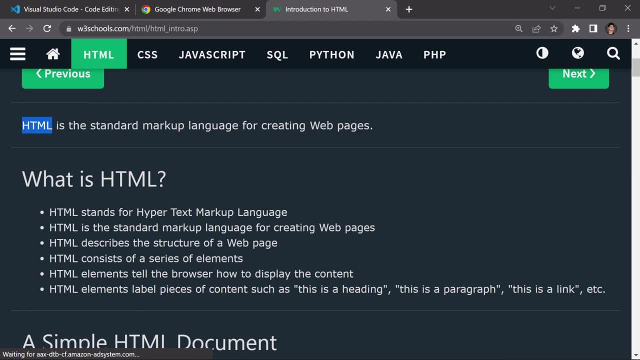 creating a website or a github account. justrov. what is html? html is just a standard markup language for creating upper functional الإيifs. in javascript is a custom format. html, html at html, that's what our lines are. allWell, you can web pages, okay, so html is some sort of a language which allows us to create a web pages. so what are? 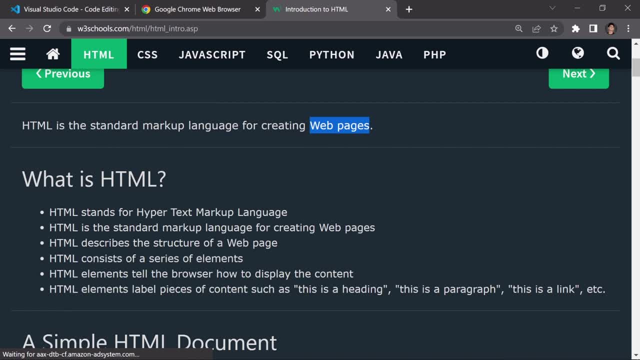 we doing in here? we are here to learn about web development, and html is our first step to learn web development. so html is a standard markup language for creating a web pages. you just have to remember this sentence right here. and the next sentence you have to remember is that html stand: 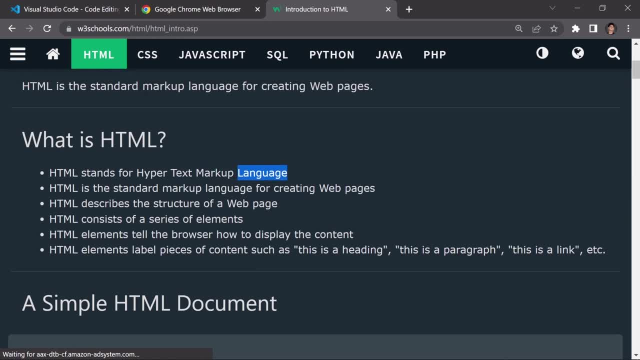 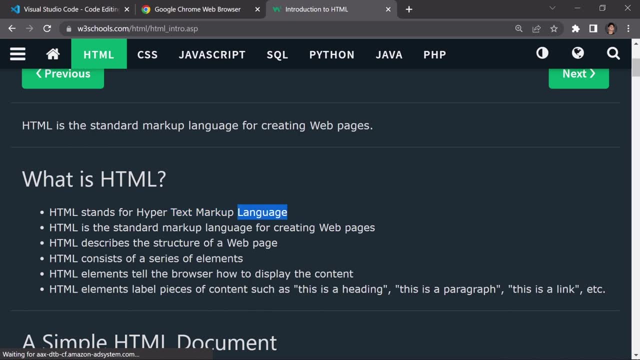 for hyper text, markup language, so that h stand for hyper, that t stand for text, that m stand for markup and then that l stand for language. so you just have to remember these two sentences: like the html. like html is a standard markup language for creating a web pages, and then html. 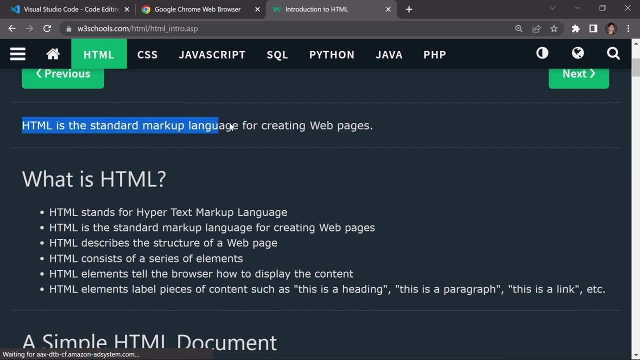 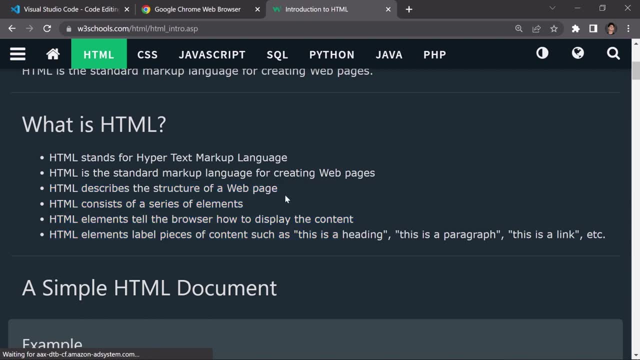 stand for hyper text markup language. so for now, i want you to just keep these two line in your mind. you don't have to care about all of these crazy terminologies like html, describe the structure of your web pages and blah, blah, blah, which i'm going to show you in this video. you don't have to worry about all of 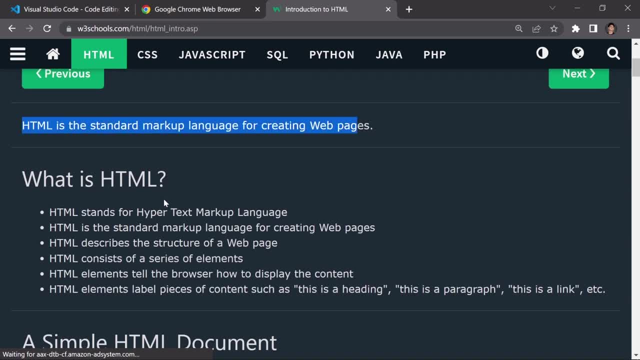 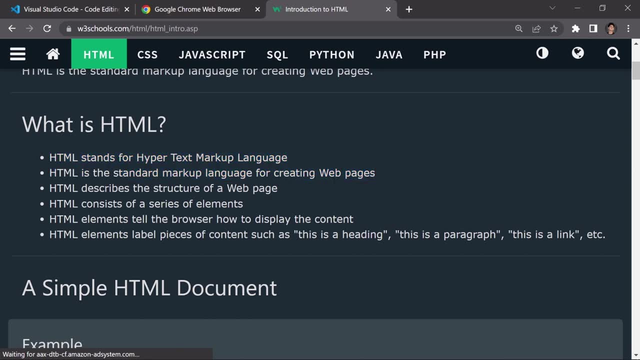 them for now, but i want you to just keep in mind these two sentences, or to be precise, like these two: html stand for hyper text markup language. html is a standard markup language for creating a web pages. okay, so this was just quick introduction about what html is, and then like: uh, what html? 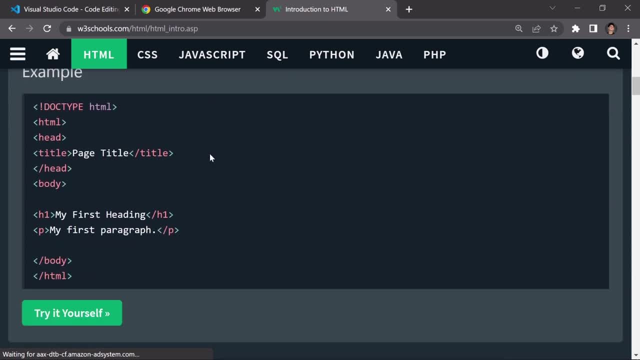 stand for. okay, and here is just a simple html document if you want to work with html. so this is first of all. you just have to remember this structure. and i know you might be thinking like, oh my god, this is a lot of stuff, like, first of all we have doc type, then we have html, head title and all of these stuff. but 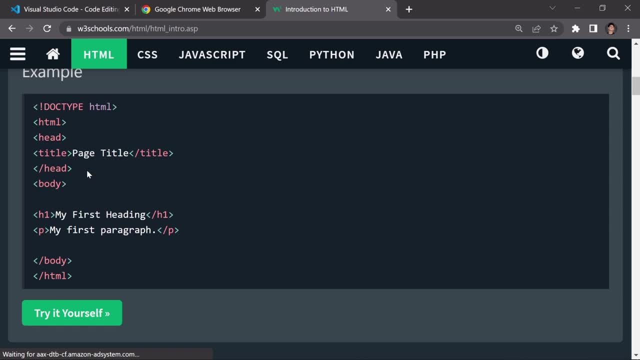 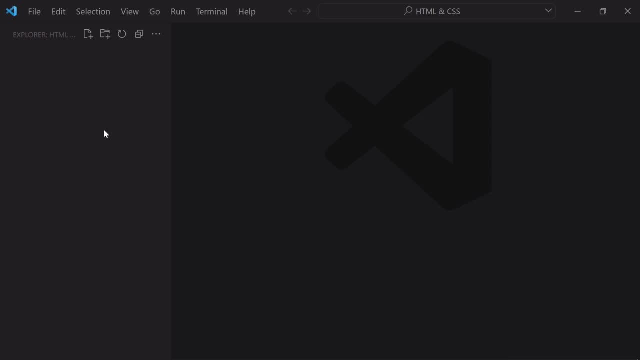 you don't have to worry about any of them for now. so first of all, let's just go to a registry recorder one more time. and now here: first of all, i want you to just create a folder. and now here, i want you to just create a new file. so if you want to create a new file in a visual story coder. 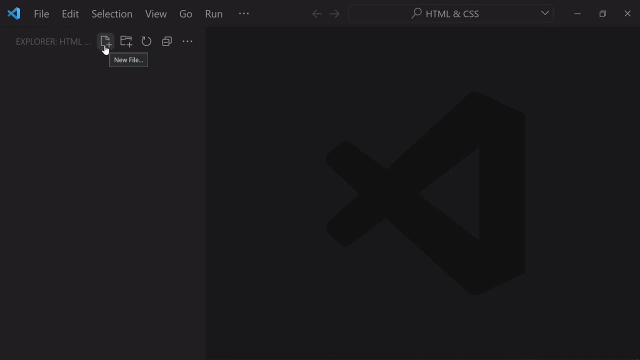 you just have to click on this file icon right here, so hover your mouse over to it and it will: new file. so if you just click on that and it will now gives us this input box right here, so inside this input box we can write uh, like the name of your file. so in this case you can give: 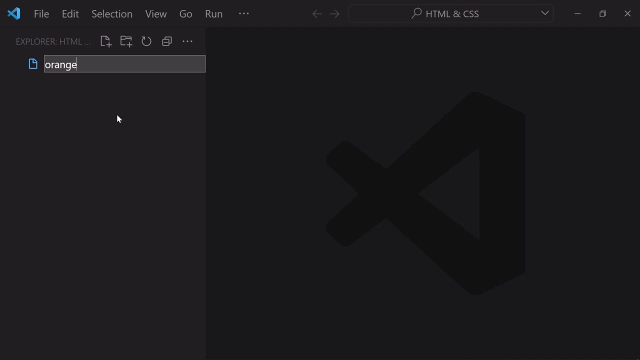 any name you like, like. if you want to give a name of like orange, so you can give them orange. you can give them your own name, if you want to, you can give them like apple. you can give like any name you want, but in my case i'm going to just give them a name of like index and remember you have. 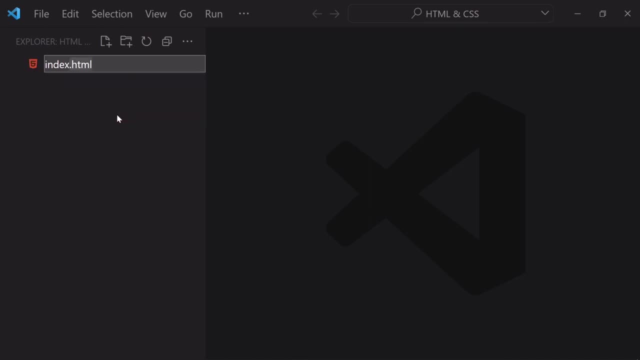 to write dot html extension. this is known as the extension, and it will tell you what to do with it, our browser, that we are working on html file. okay, so if you don't provide that here, you can see that uh, logo kind of thing is gone from here. and if you do, provide dot html- and what is html stand? 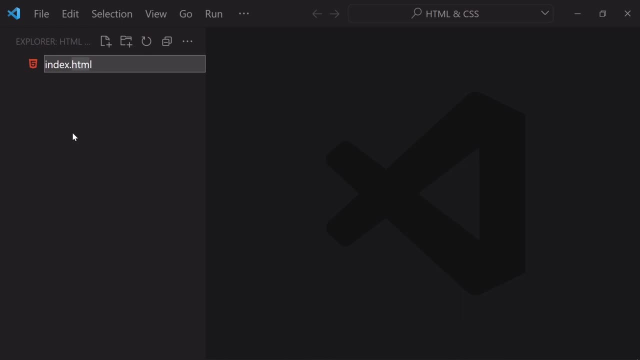 for html stand for like hyper text, markup and language. okay, so you just have to provide that. you can give any name you like, but you have to provide this dot html at the end of the file. so in this case i'm going to just write index and then dot html and now, if i hit enter, right here. 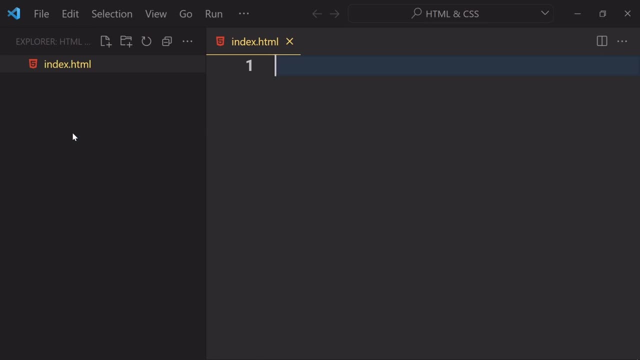 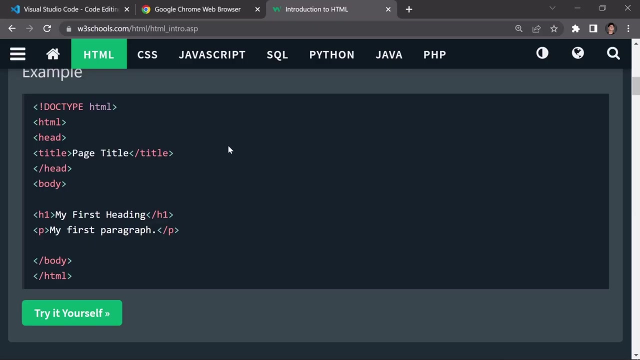 and boom, here you can see, we have our first indexhtml file. so now the next thing i want you to install in your visual story coder is something called extensions. so let me just show you that in your case, the extension look like this. so i want you to just click on these four. 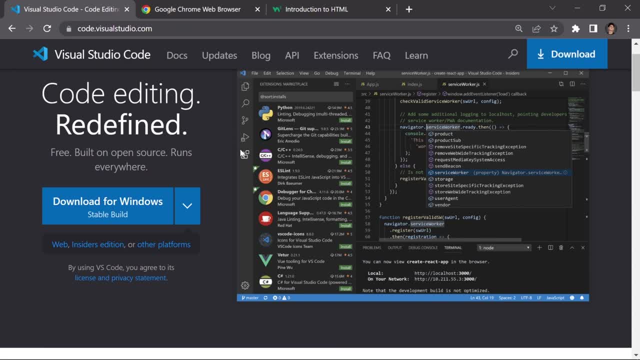 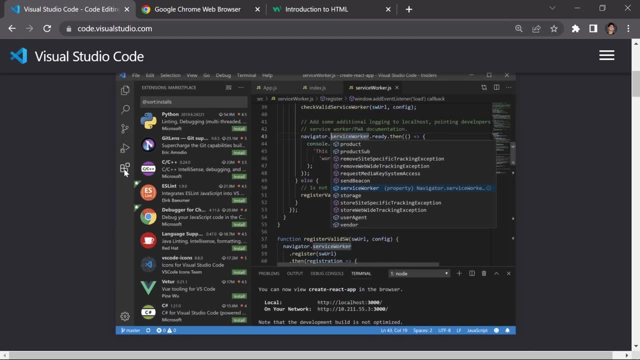 boxes right here, not this one, not this one, not that one, not this one. but i want you to just click on these four boxes. let me just zoom in a bit so you can see everything. i want you to just click on these four boxes right here. in my case, i'm going to just hold control and then i'm going. 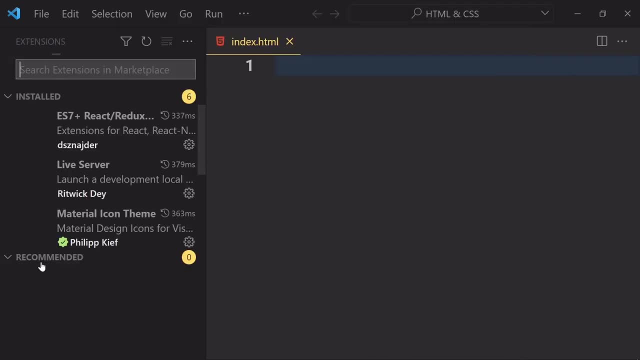 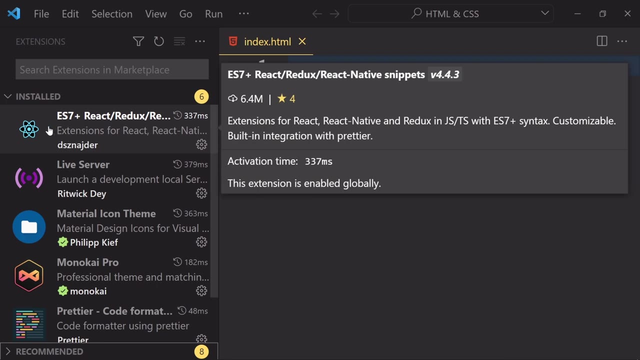 to hit key and then i'm going to just click on this extension and you don't have to do that. and now, here you can see, i have a lot of extension which i installed in my visual story recorder. you don't need to install a react extension and stuff like that, but for this course i want you. 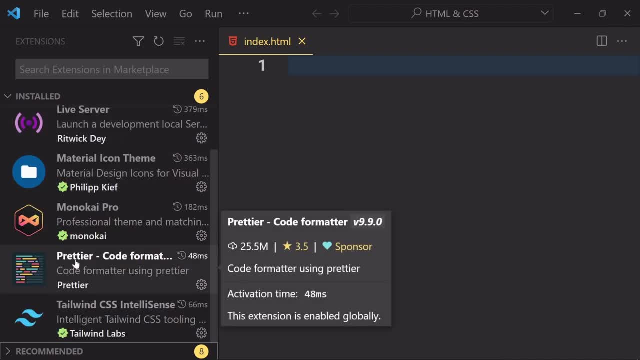 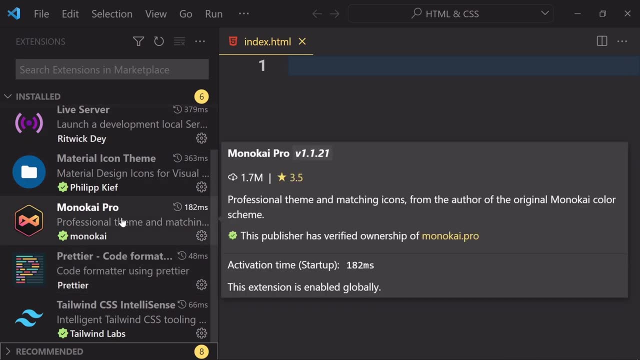 to install a live server and also this prettier, okay. so i want you to install both of them in your visual story coder. so if you also want to install this monokai pro theme, so you can also install that. but in my opinion, like you don't have to, if you want to install it, so you can. 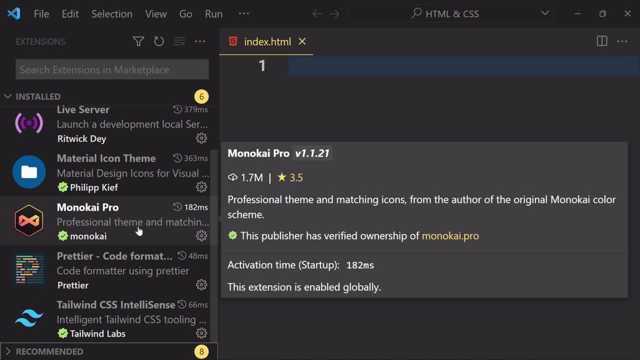 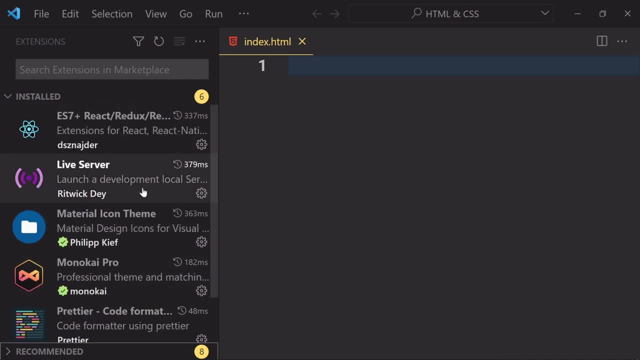 but if you don't want to install that, you just like: don't install it. so you have to install this live server for this course and you also have to install this prettier coder for this course. okay, so this is it. now i want you to install both of them like live server and then prettier extension. 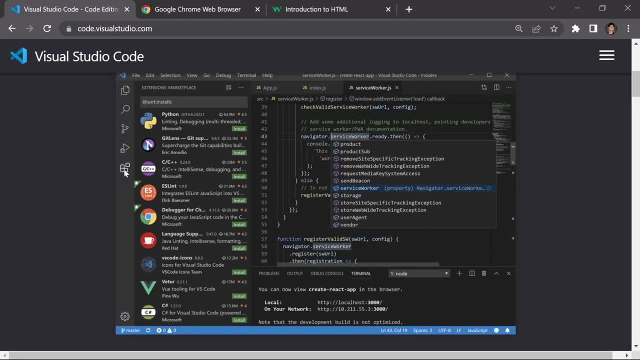 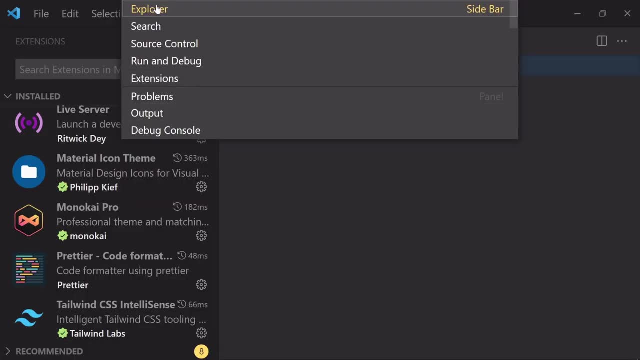 and then what do you have to do then? instead of clicking on these four boxes, i want you to just click on these two file kind of icons. so in my case, i'm going to hold control and then i'm going to hit kill, and then i'll just click on this explorer and it will now give us this indexed: 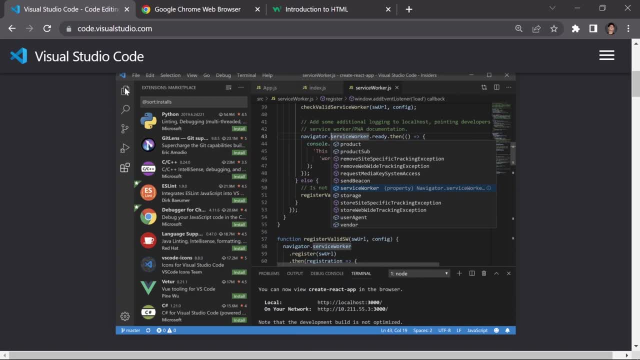 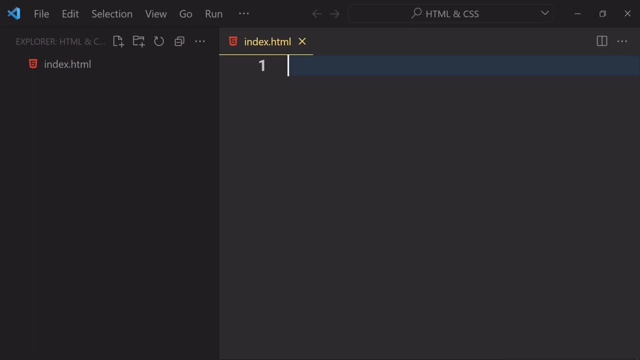 html file right here, okay, so i want you to just click on these uh, two kind of files anyway. so now we successfully create our indexhtml file, and i'm assuming that you already installed there two extension which i just show you now. the next thing which you have to do is that you have to hit. 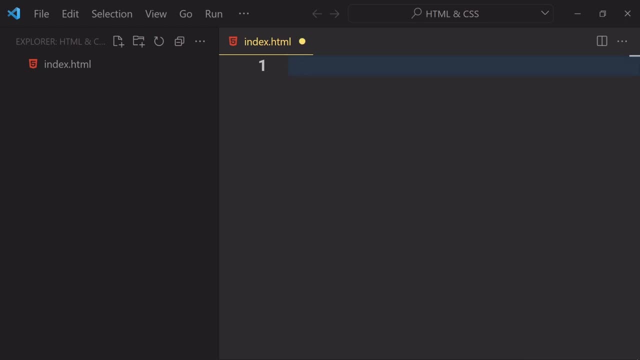 control and then a comma. okay, so i want you to just hold your control key and then i want you to just hit this comma right here, not a period, like not this dart, but i want you to hold control and then hit comma. so if i just hold control and hit comma, so here you can see it. unlock uses the. 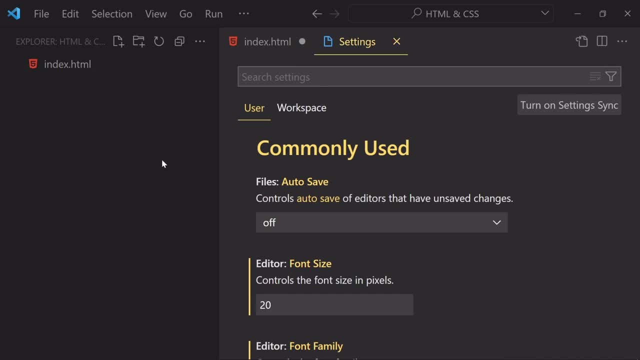 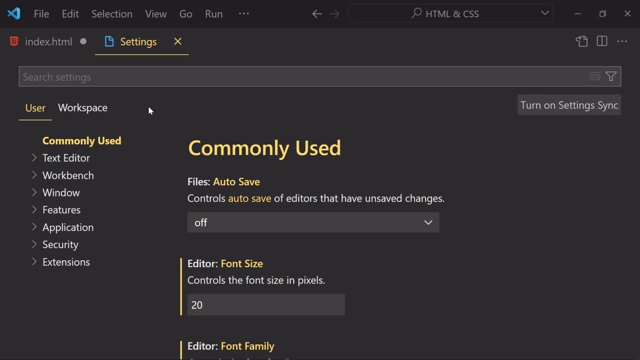 settings right here and now. if you want to remove this sidebar from your eye, so you can just hold control and hit b and it will now remove that if you hit control, if you hold control and hit b one more time, so it will now show it and hide it like that. okay, so now, here you can see we are now at. 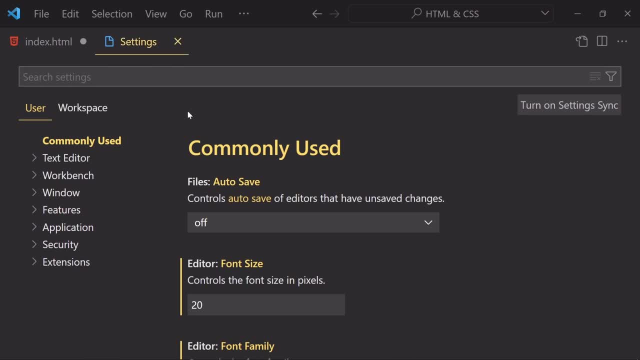 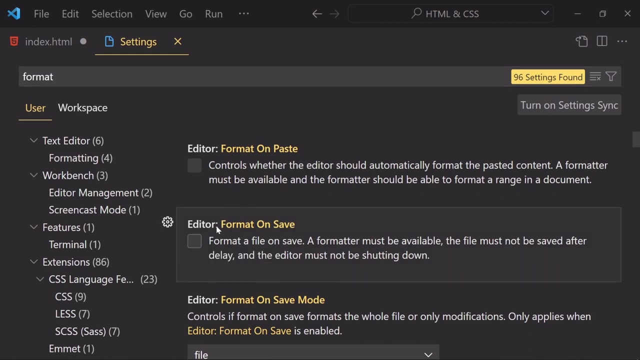 the setting right here. now i'm assuming like you've already installed that two extension in your registry coder. so what do you have to do? you just have to type like f-o-r-m-a-t, and then here you'll find an option like format onset. so by default it will be set to uncheck. and now i want you to just click on this check so it will. 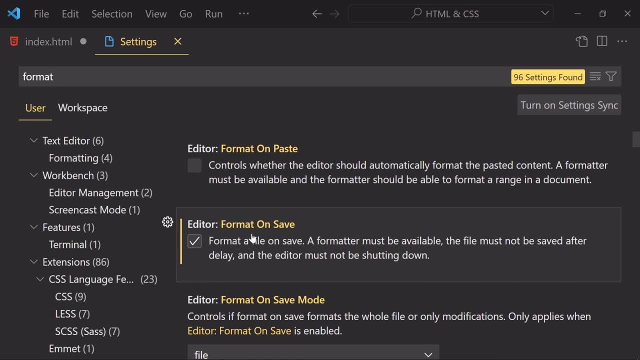 just install or not install, like any, any time you save your file, so it will just format your document and you don't have to worry about saving and all of that crazy kind of stuff which i'm saying right now, which i'm going to show you everything just like one by one. and now i want 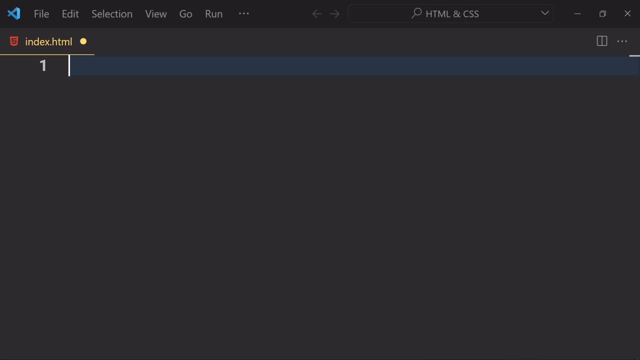 you to just click on this x, so now it will just remove that anyway. so i'm going to just zoom in a bit and you don't have to zoom in if you want to zoom in or out in just recorder. so you just have to hit control and then hit plus, so it will just zoom in. and then if you hit control or hold control, 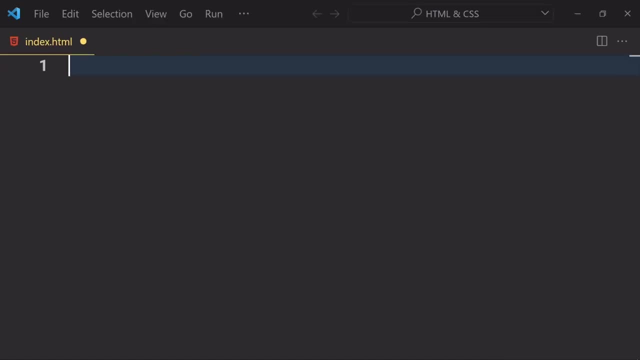 and then if you hit minus, so it will just uh, minus or zoom out. okay, so this is how you can zoom in and zoom out in which is recorder. so now the first thing i want you to notice- and i'm going to also hide that sidebar and you don't have to. 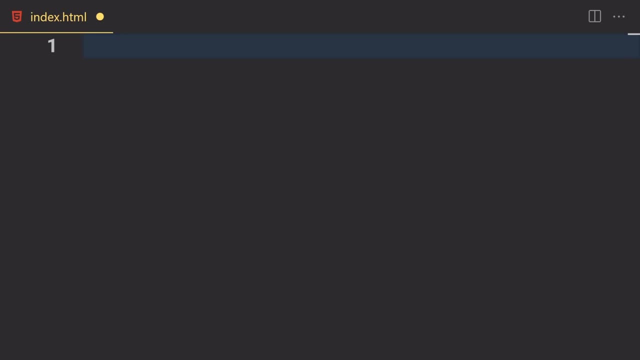 so the first thing i want you to know is the structure of html. so what is the structure of html? first of all, let me just tell you like html structure can be a little bit horrible at first if you see that, but trust me, it's not that. 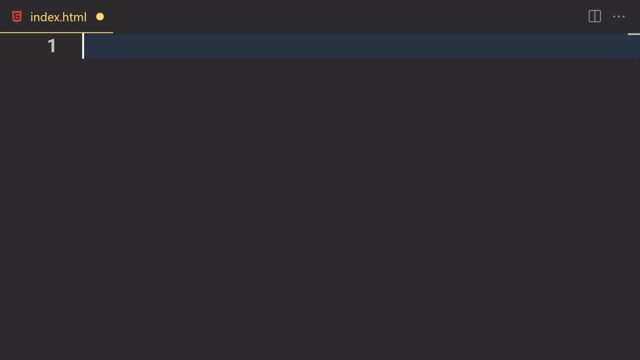 much like hard to learn. it's a very easy thing to learn, okay, so you just have to first of all write a less than sign and then this explanation mark, and here you can see visual story coder is already helping us. like: uh, do you mean like doc type html? yeah, we do mean dog type html. so if you click on 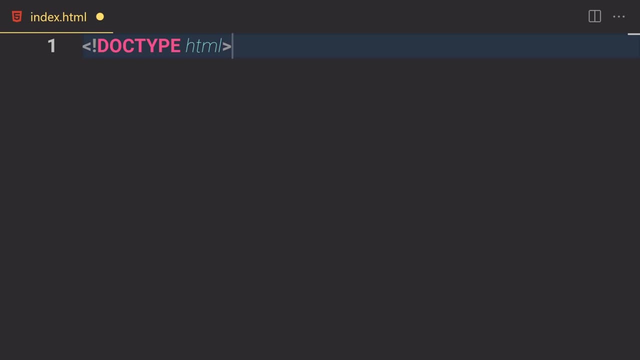 that, and here you can see it, will not auto complete it for you. so first of all, i want you to write this explanation mark. so if you want to write this symbol like explanation mark, so you just have to hold shift and then hit one. so here you can see it will. now gives us that explanation. 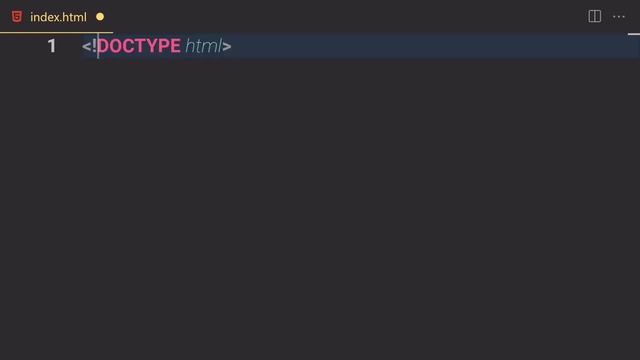 mark right here. i'm going to remove that. so first of all let me just say that one more time. you just have to write a less than sign, then this explanation mark and then uppercase doc type. so you just have to write that uppercase. you cannot type there like a lowercase dot type. it's not a. 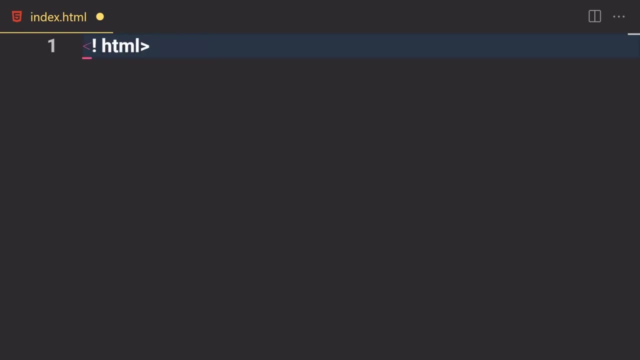 valid syntax. you have to write that in uppercase, so you're going to be writing like d or c, t y, p, e, okay, so here you can see it now highlighted as red, and then in lowercase you just have to write html and you don't have to worry about like: what is this doc type? html will do for us, which i'm 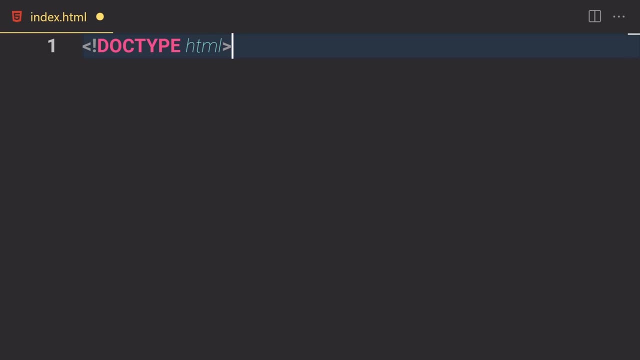 going to tell you in a second, but you don't have to worry about it for now. so i want you to remember that anytime you want to work with the html, first of all you have to create your file somewhere in your machine, and now the next thing which you have to do is that you're going to be writing this: 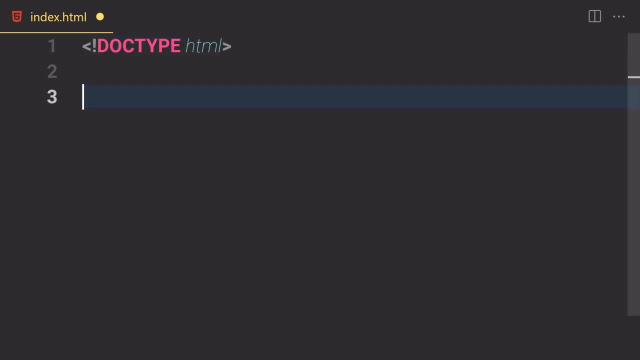 doc type html. so these are important stuff. now, the next thing which you have to do, the next thing which you have to do is that you just have to write html, and if you are using a visual story coder, then i want you to just hit tab and it will auto complete it for you. okay, 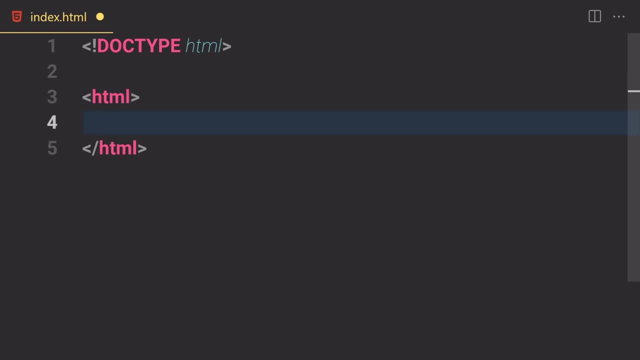 and then i want you to just hit enter. and now here you can see the log, users or root tag right here. like we have html opening tag and then we have html closing tag. now you might be thinking like, what is the opening and closing tag? anytime, you want to work with the html tags, first of all you 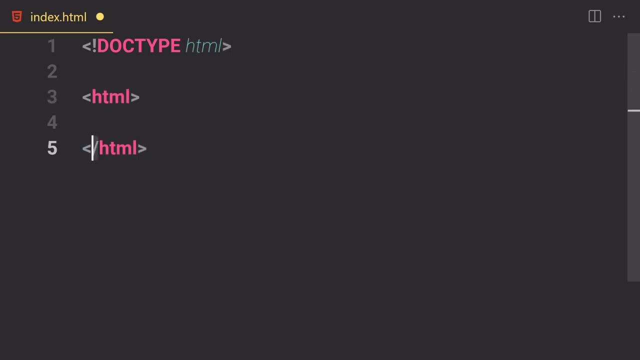 open that and then, if you want to close that, you would just write this right here at the end, so it will now just close it for you, okay? so here you can see. we have a dog type html, then we have our html opening tag, and then we have html closing tag and we are going to 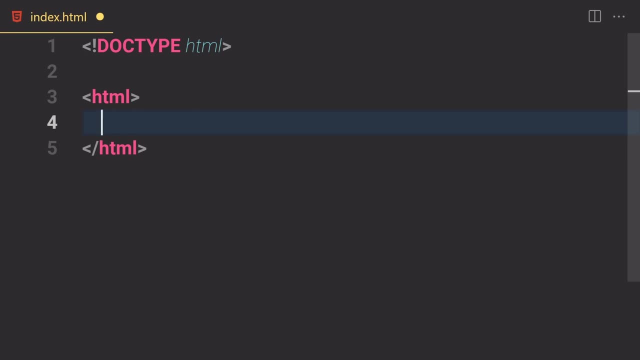 be also learning about something called a self closing tag, which you don't have to close, which will just close itself. okay, you don't have to worry about all of that for now, but i want you to just remember. first of all, we are going to be writing a dog type html, then we are going to be 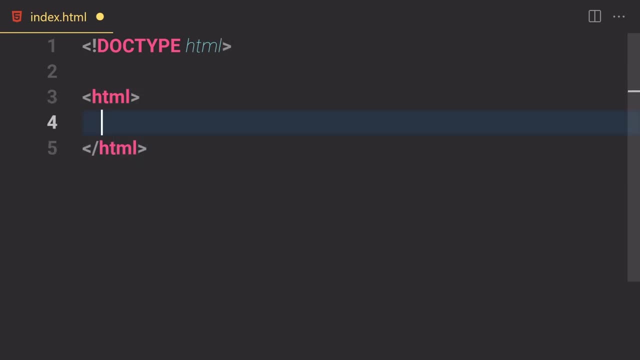 writing html opening tag and then html closing tag. and now inside this html, what do we have to do? we have to write another tag, which is known as a, h, e, a d. okay, and if you're using a visual story coder, you just have to hit tab. and if you are not using a visual story coder? so what do you have to? 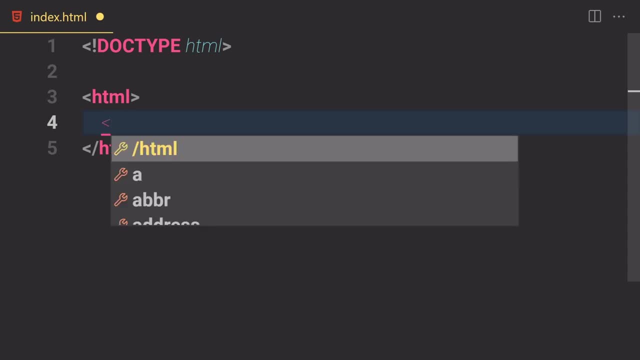 do? first of all, you have to hold shift and then the less than sign, and then you have to write manually like h, e, a, d, and then you have to write a greater than sign, and here you can see my visual story. coder will help me auto complete it for me, okay, so first of all we have a html, then inside. 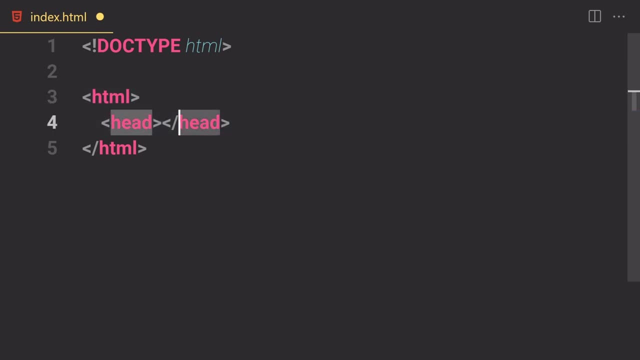 this html: we have a head opening tag, and then we have a html closing tag, and then we have a html closing tag and then head closing tag right here. so here you can see, we have this slash right here, which means like closing tag. now what do we have to put inside this head area? well, we just have to write our. 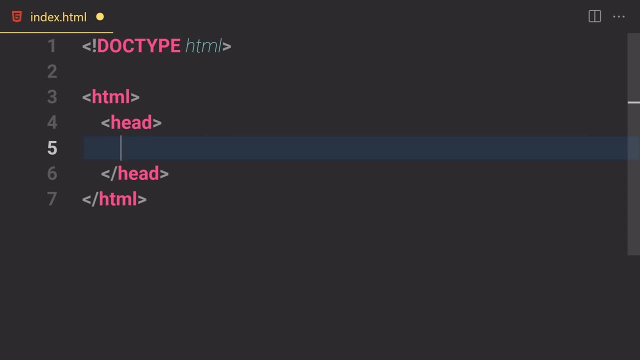 title. okay, so i'm going to just put like: for now i'm going to just write like t-i-t-l-e, and if i hit tab right now, so it only gives us title opening tag and title closing tag right here. okay, so anything we put inside a title area will show up at the top of our page. so in this case we are going. 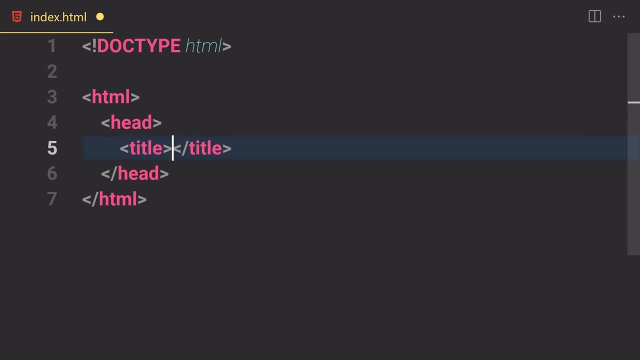 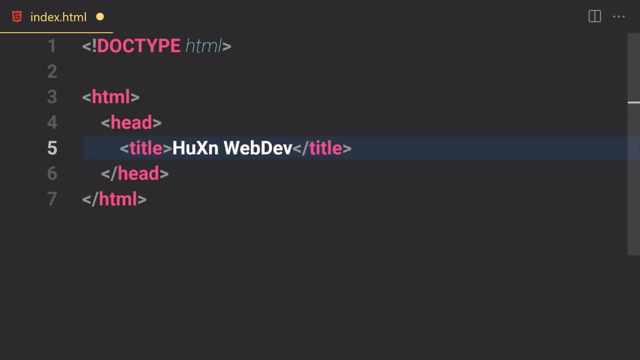 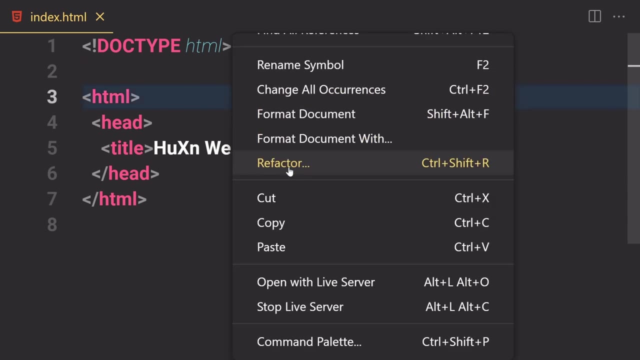 like h-u-x-n-w-e-b-d-e-v. so hosan, webdev and knife is cell file, so i want you to just right click on anywhere inside your html document, then i want you to just scroll down and here you'll find this open with live server. and remember, this option will be only available if you already 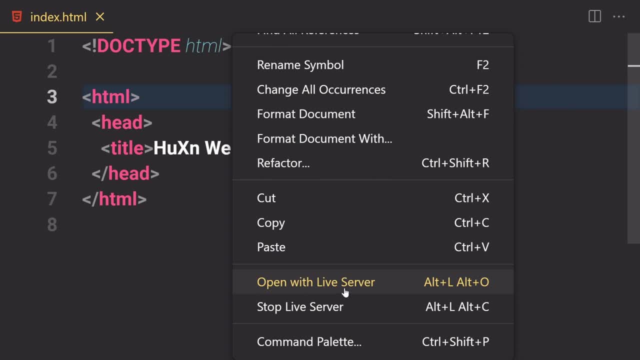 installed live server extension in your machine. if you did not, then i'll suggest you to install it first of all. so then click on this, open with the live server, and it will now open your file in a live server just in a second. and now here you can see, it will now open our file in. 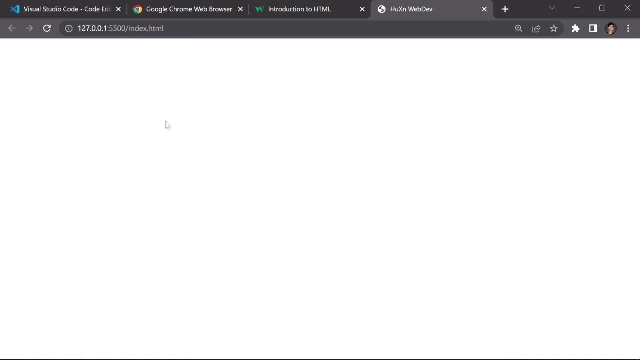 live server and now it's totally blank at the moment. now you might be thinking: like we already write our name right here, like hosan webdev, right here. where is that located? well, you can see that right here, like we have this hosan webdev, if you just remove that. and we didn't provide anything. 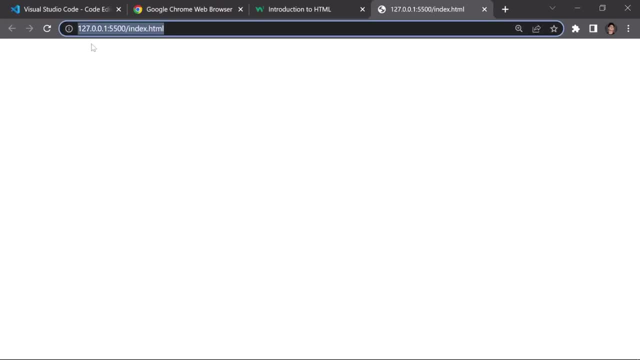 and if you just save our file, so here you can see, it will take this link and it will put it right here. so here you can see, we have this kind of a long name which will come by default once we install a live server. so live server will help us, uh, by providing this 127.0 and stuff like. 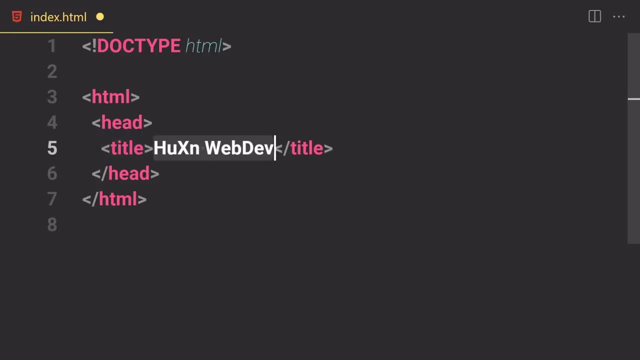 that okay. so we have to provide, like some sort of a title for our page, and then now the next thing which you have to remember is something called a body. so if you just write a body and if you hit tab, certain log users like body opening tag and body closing tag right here and it will not be. 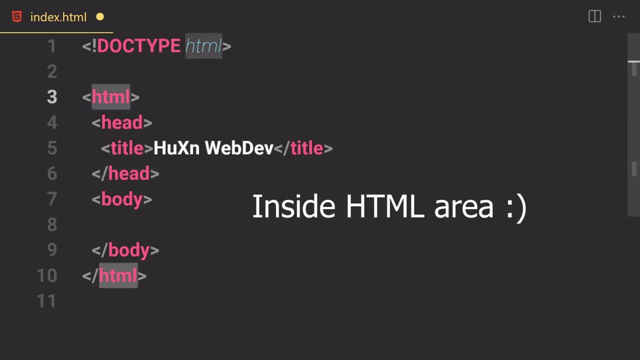 inside a head area, it will be inside a title area. so now let me just put that right here so you can see it a little bit better. here you can see, we have first of all a dog type html, then we have html opening tag, and then the html closing tag, and inside this html we have a head opening tag. 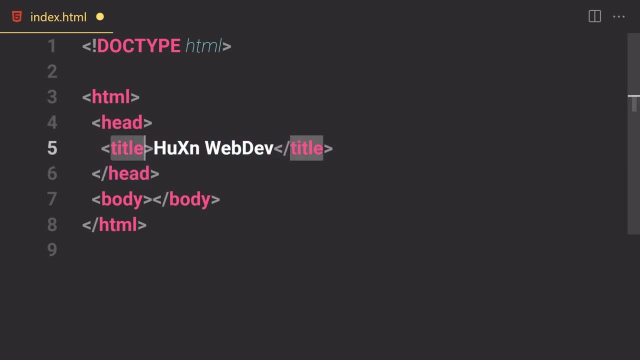 and then head closing tag and inside this head area we have a title opening tag. then we have some sort of a title and then we have a title closing tag. then outside from this head area we have a body opening tag and then body closing tag, right here, and anything we write inside this body. 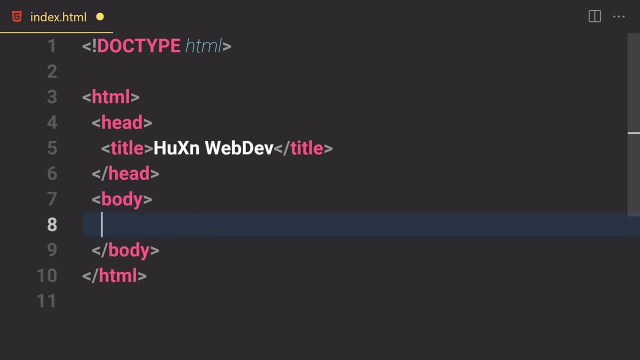 except comments, which we are going to be learning very shortly. so anything right inside this body will show up to the user. so in my case, i'm going to just type some gibberish right here and you can write your own name or whatever kind of text you like. and now if? 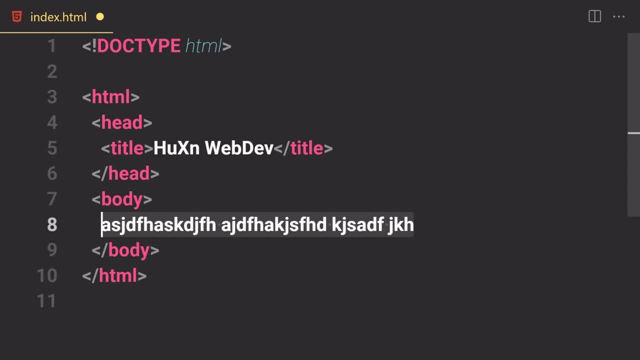 you save there and, by the way, you have to remember these seven things which i'm talking about. so if you didn't save your file now, let's suppose we just write this kind of our gibberish, or you know, i'm gonna just put my name. and if you just write there and we didn't save our file, and if you go to 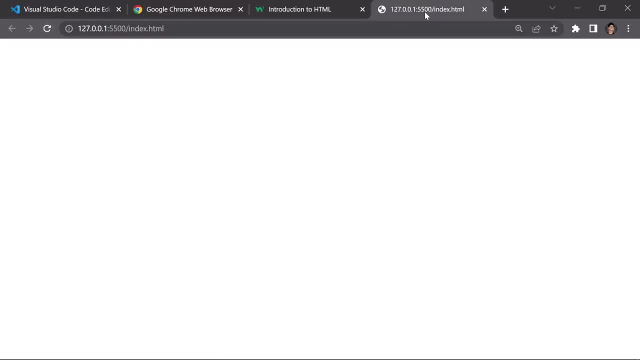 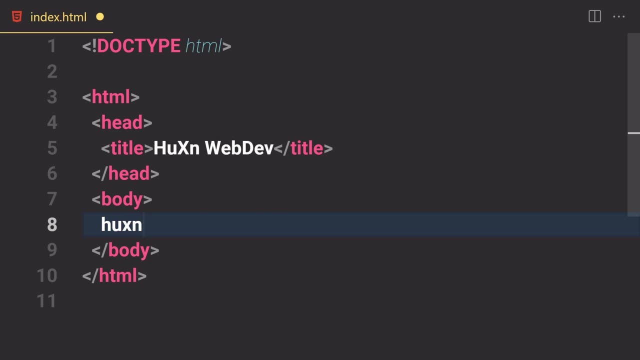 our browser and if you refresh, nothing will show up right here and also right here. why is that going to show up in your browser? okay, so the problem is that we just uh, saved our code and then hit save, and if your browser will switch to save our code, then it will take red書 and 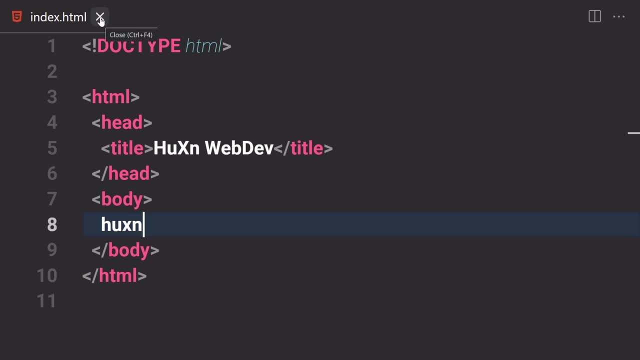 it will work as if it is saved our external code. so if your browser is not receiving doozies, in your browser it will just have itàyавы infinito to save your code. but we didn't save our code in your machine. so if you want to save your file, so first of all you just have to hold ctrl and then hit s, so it will save your file. and now here you can also notice that we have this circle right here. if you just write a space, it will also gives us the circle right here. it mays that you didn't save your file and it means that you don't save your file if you only save this file. 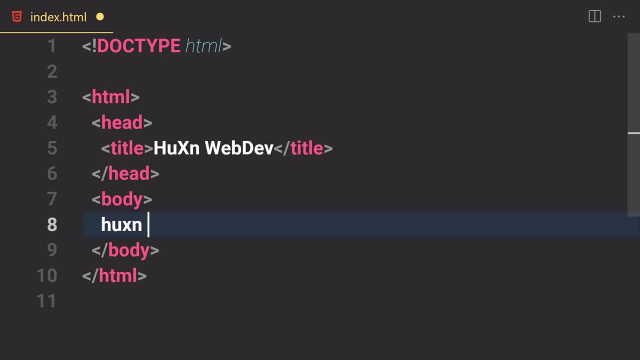 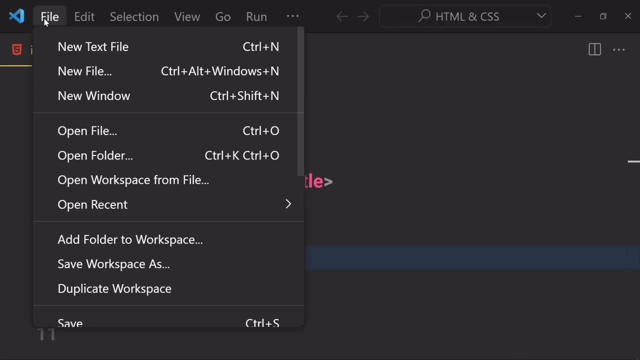 it means that you have to save your file. so if you want to save your file, so you can just hold control and hit s button so it will just save your file. or you can just click on this file and then just scroll down and here you would find like a save, and save as a kind of a buttons right. 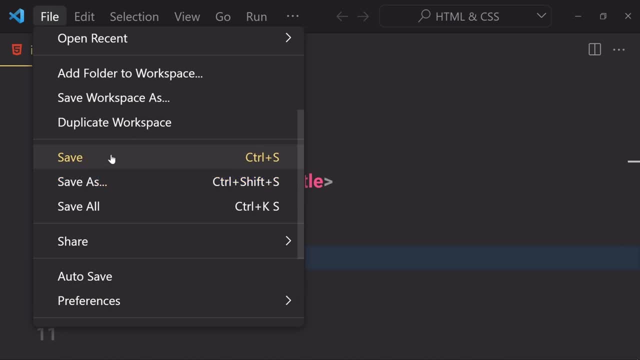 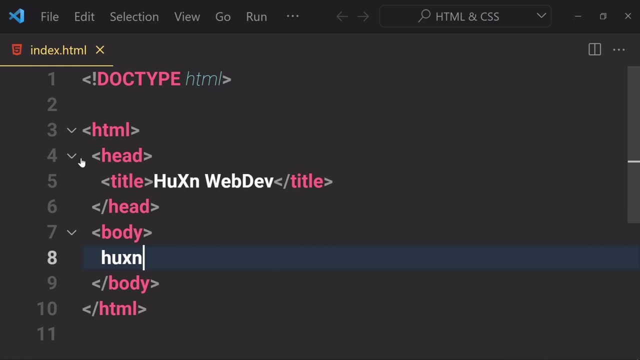 here. so save will allow you to save your current file, and save as will allow you to save it to somewhere else. okay, so i'm going to just click on this save one right here, and if we check our browser, so here you can see we get huzzan right here and, as i said, anything we write inside this. 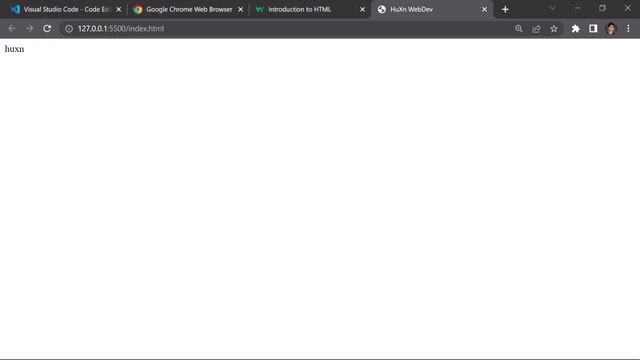 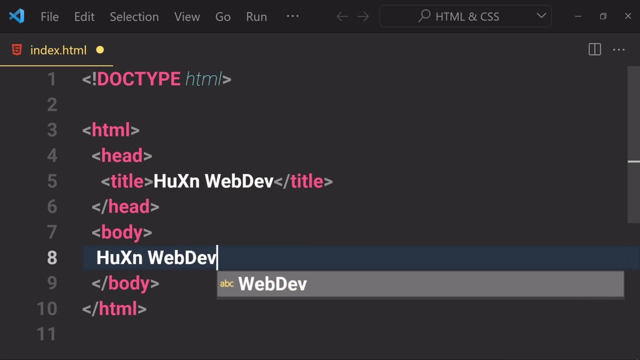 body area will show up to the user. so this is how we can see our huzzan right here. so now let me just write something else, like in my case i'm going to just put like huzzan and then webdev as well, and now, if you didn't save our file. so here you can see, we get this circle right here and now. 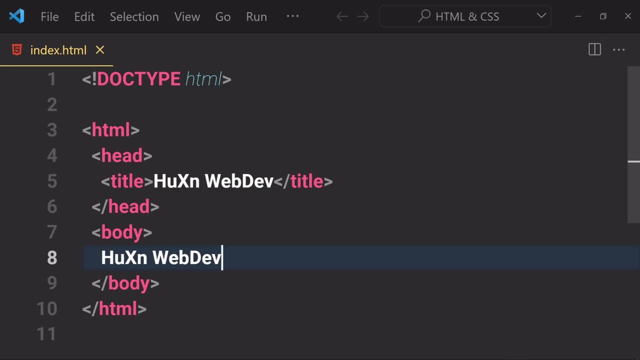 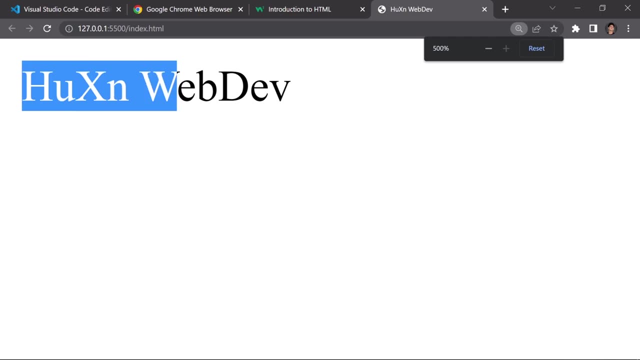 if i want to save my file by holding control and hit s. and now, here you can see, that circle is replaced with this x. right here, okay. so here you can see. we are now getting the huzzan webdev inside our body. right here, okay. our web page, to be precise. and in this course, i'm 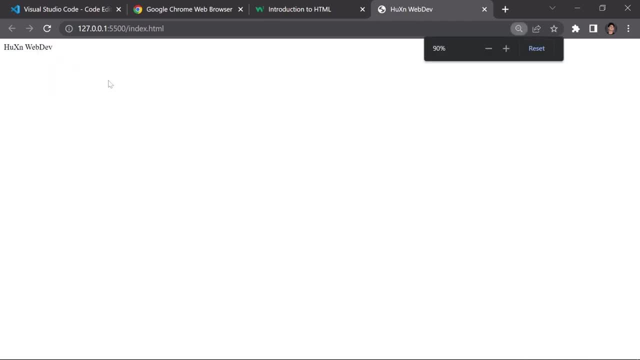 going to be zooming in and zooming out so that you guys can see everything a bit clear. so if you want to zoom in and zoom out at the same time so you can just hold control and then inside your mouse you can just scroll in or scroll out, okay, so scroll in will allow you to zoom in and then 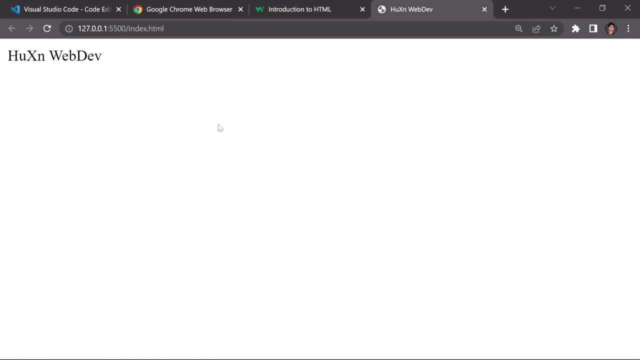 scroll out will allow you to just zoom out, or you can just also hold control and hit plus, plus, plus, plus, so it will just zoom in, in, in. and you can also hold control and minus, minus, minus, minus, so it will just zoom it out for you and the default size will be just 100. so the default size will be just 100 it. 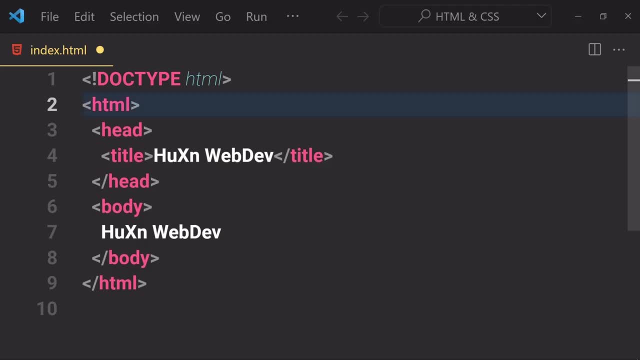 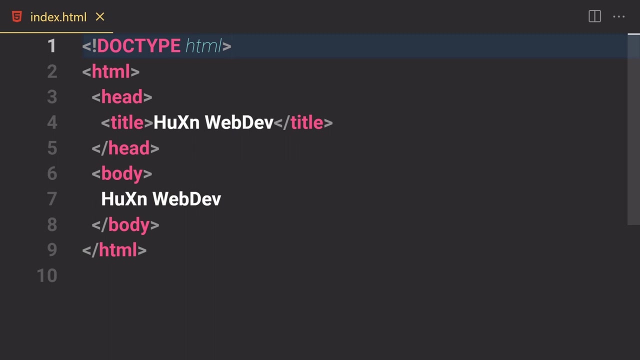 will look like this. so, now that we're totally done with our structure, right here the structure of html, and this is how the html structure look like. now let me just explain all of them one by one. okay, so first of all, we have this doc type, html, and this is also known as a dtd and dtd just. 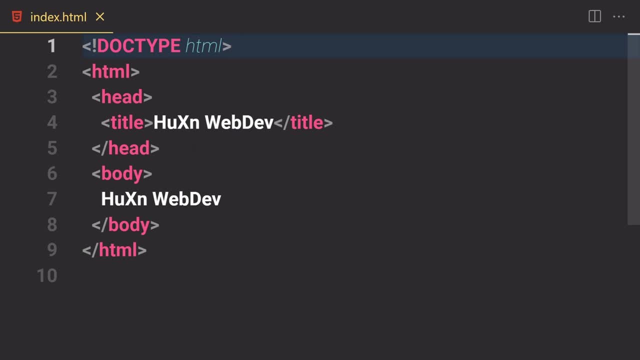 stands for, like, document type declaration. i know these are a lot of words, you don't have to worry about any of them, but i'm just saying, like for those people who are interested in this theory, kind of stuff. so this doc type html will just tell our browser that we are working on a html5 document. 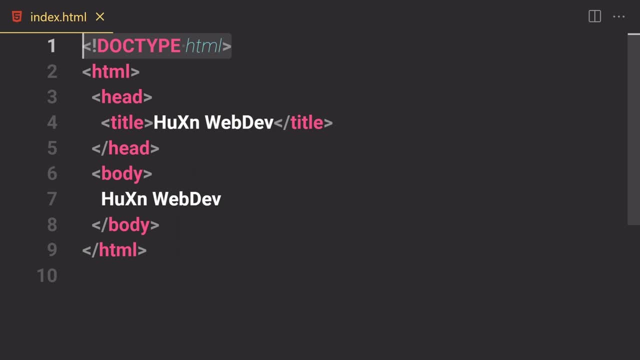 not html4, not html3, not html2, not html1, but we are working on html5. so what is html5? html just stands for like hypertext markup language, and it is the fifth one: html5, html5, html5, html5, html5, html5. 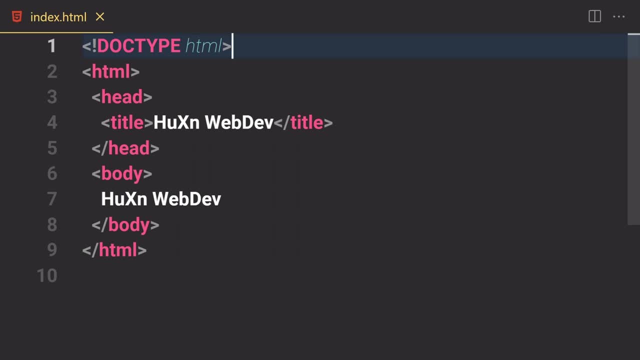 fifth version of html, okay, and this version allows us to put a video and audio files as well inside a browser. then we have a root tag. so here you can see, we have html opening tag and then html closing, and these are also known as a root tag. okay, because these will be the 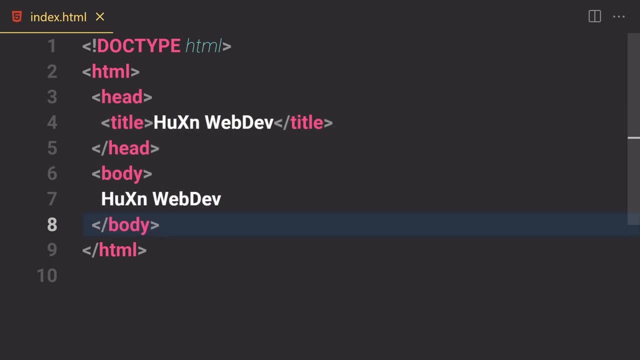 root of all of our coding. then we have a head area and inside this head area we are going to be putting our metadata- like we are going to be putting metadata later, but you don't have to worry about metadata for now- and we are going to be also linking it with our css. 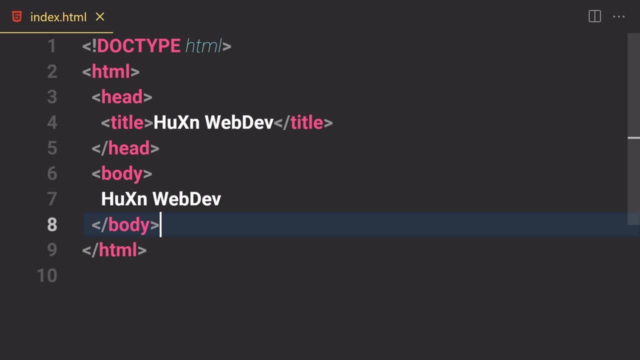 files and javascript files and stuff like that, but you don't have to worry about all of them. for now as well, the title- and you already saw like what a title will do for us, and as the name suggests that it will be the title of our web page, and here you can see we have the title of 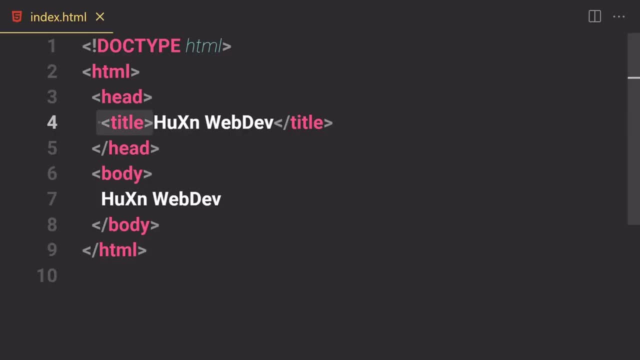 our web page right here, okay. and then the final thing, and as itself says, like we have a body area and then body just stands for like a body, you know. so in anything we write inside a body will show up to the user. it doesn't matter if you just write like one, two, three and stuff. 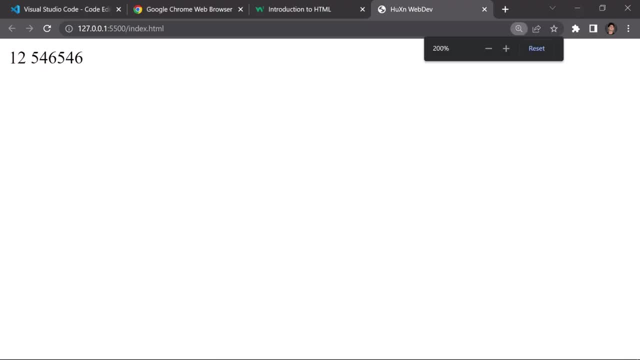 like that. so if you save our file and here you can see we are now getting these numbers, and if you just write some gibberish like i don't know, and if you just save that and here you can see we are now getting these gibberish right here and in and we are going to. 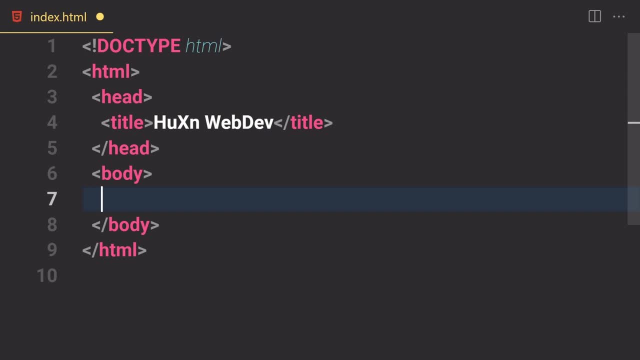 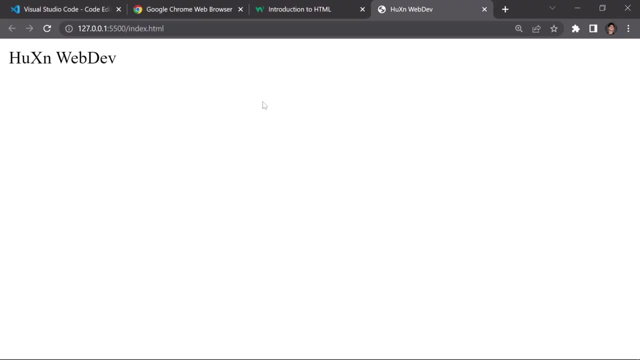 be writing a lot of stuff inside a body area. so this was kind of a theory you can say, and now in my case, i'm going to just put my name like huzzain web dev, and now if you sell a file and boom, we get a huzzain web dev right here inside our browser, and so this was kind of a structure of html and 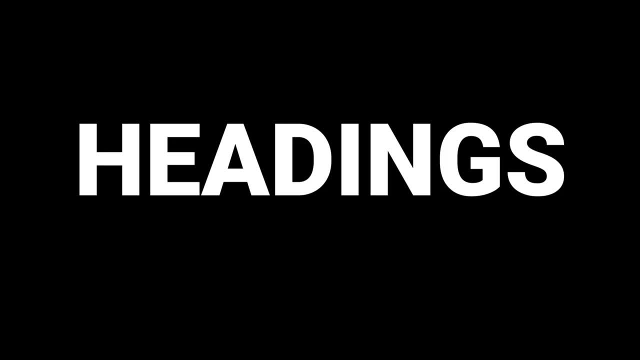 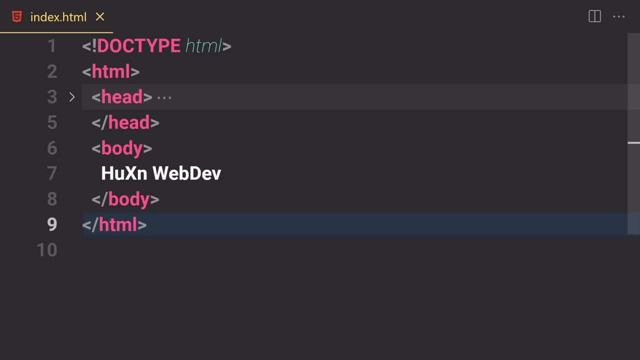 how to set up your machine for writing your coding. all right, so now that we know enough about the structure of html, so now the next thing which we are going to be learning is something called headings. in html, headings are just a main title or the subtitle of your page. okay, and in html, we have headings from h1 through h6, like we have h1. 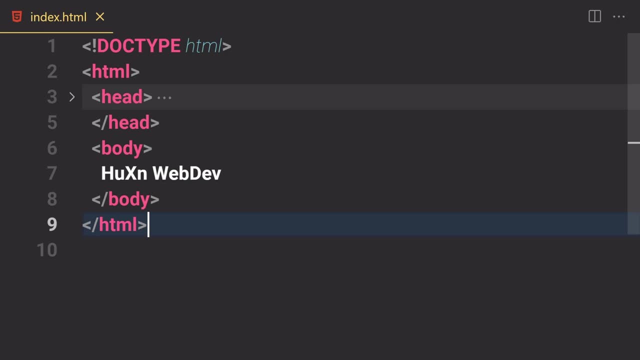 h2, h3, h4, h5 and h6. okay, so first of all let me just write some code, then you'll get to know what headings are. and now i'm going to just remove my name from here and i'm going to just write like: h1. 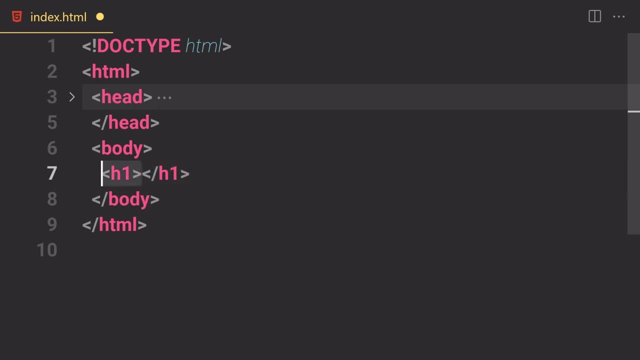 and i'm going to hit tab right here. so what do we get? we get like h1 opening tag and we also get h1 closing tag right here, and anything we write inside there will be our first heading, okay, and this one will be the top or the best heading of our page. or you can also select the. 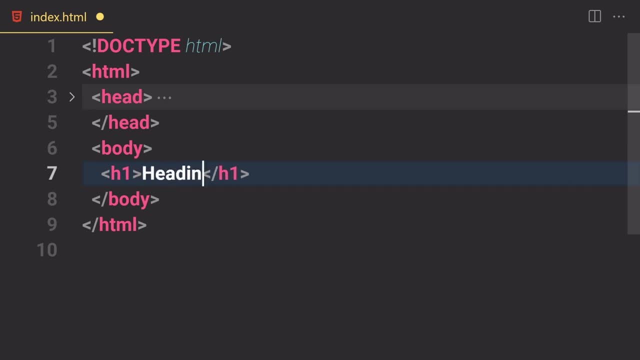 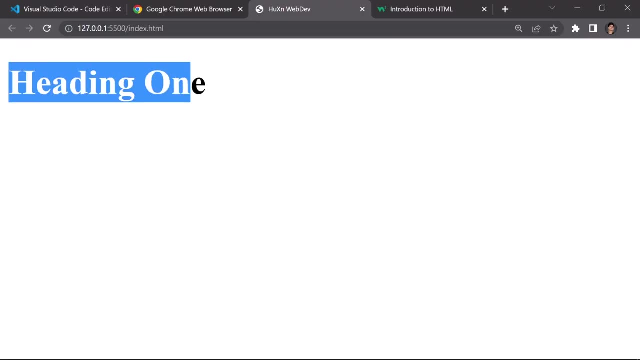 main heading of our page. so in this case i'm going to just write like heading and then one. and now, if i send my file and if i preview that and here you can see, it unlock uses these huge heading one right here. okay, so i guess i resumed in and this is how it will look like by default. 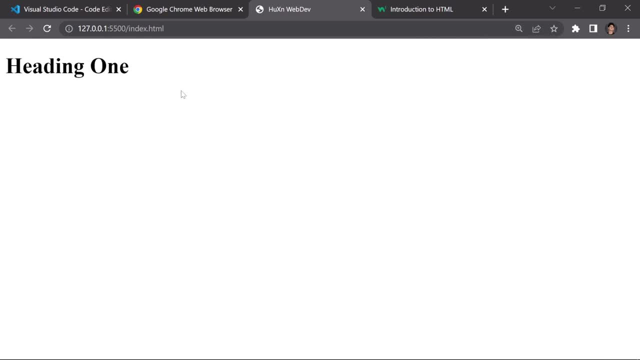 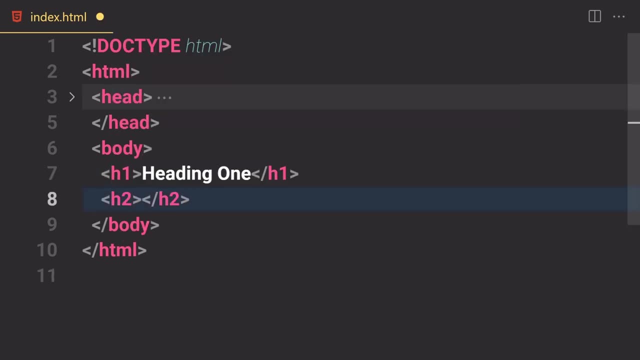 okay, so now i want to just zoom in a bit so you guys can see everything a bit clear. so this is h1, like heading one, and now if you just write like h2 right here, and if you had tab, and now here you can see the log users. h2, right here, like heading two, and now if you just write like 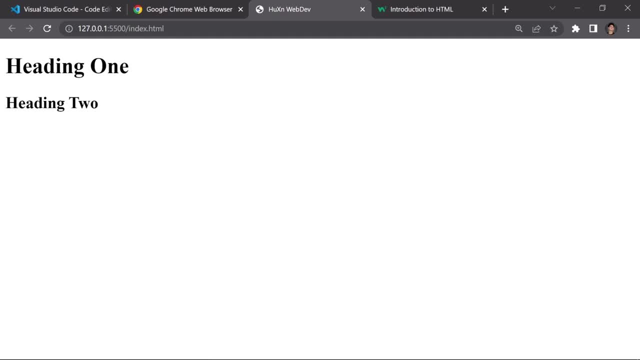 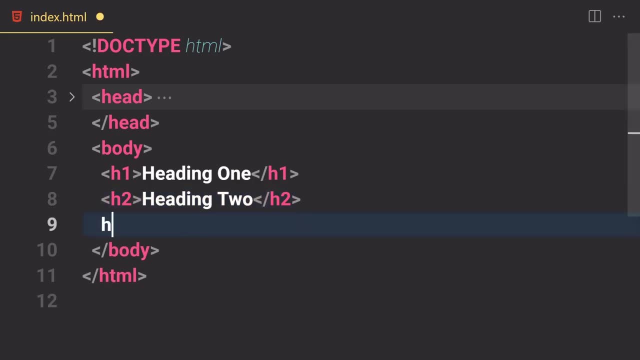 heading two, and if you save that, and this one will be a little bit smaller than the first one because this is the subheading or the second heading of our page, then we have three. so now let me just write h3 in here, and if you hit tab and now it will gives us heading three. 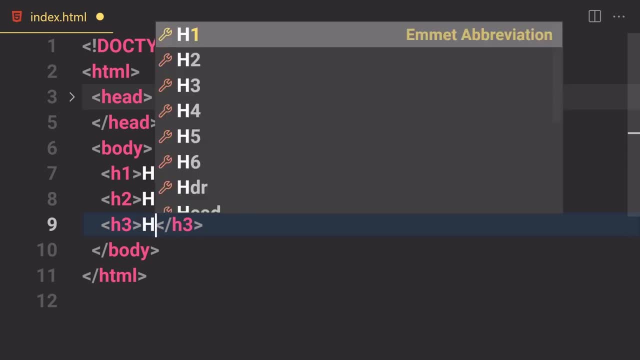 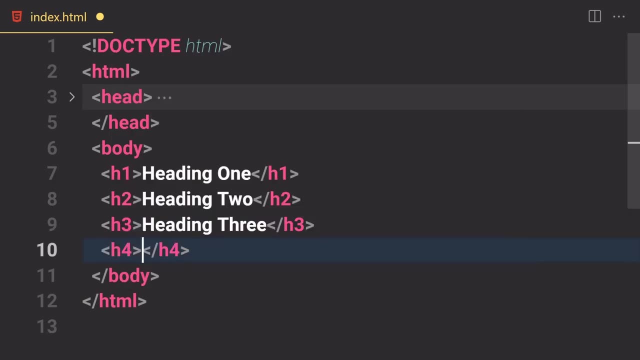 opening tag and heading three, closing text. so i'm going to just write like: uh, heading three in here, uh th r double e. so we have heading three. then we we are going to be writing h4 of heading four and then h5 of heading five, and let me just write like heading five to lower case. and now let me just 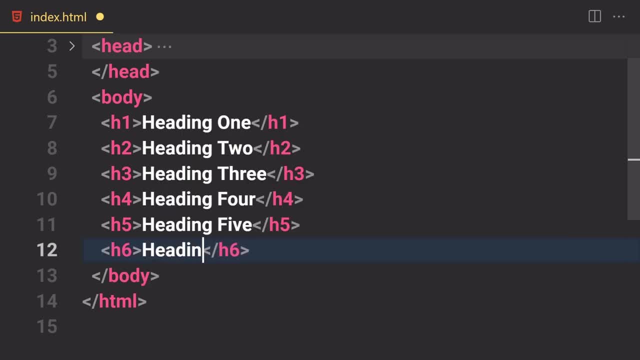 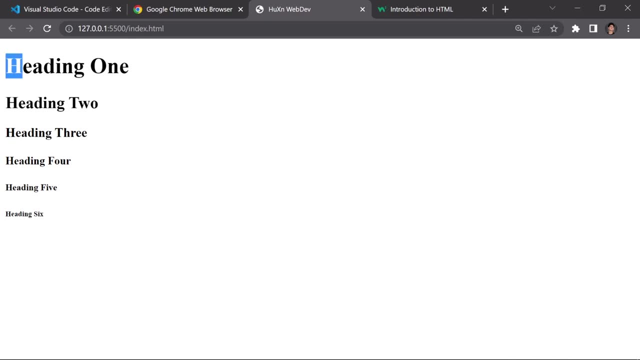 and this one will be the final one here. i'm gonna just put like heading uh, six right here and now. if you just save our file and boom, this is how it looks like. so the first heading we have is h1, and this one will be the best heading right here. then we have h2, h3, h4, five, six and so on, and so 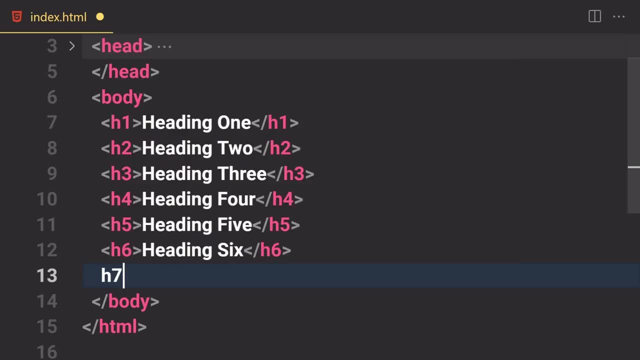 forth. and now, if you try to write like h7, if you just write h7, if you hit tab, it will not gives us any code completion. why? because we don't have h7 in our html, so that's why, or we just recorded it is not helping us in this case. so now, if you just try to write it like manually, like if i just 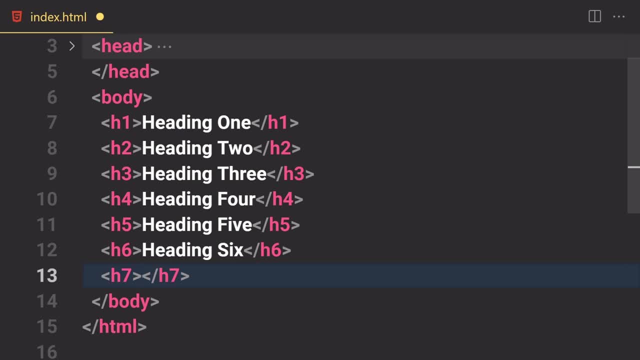 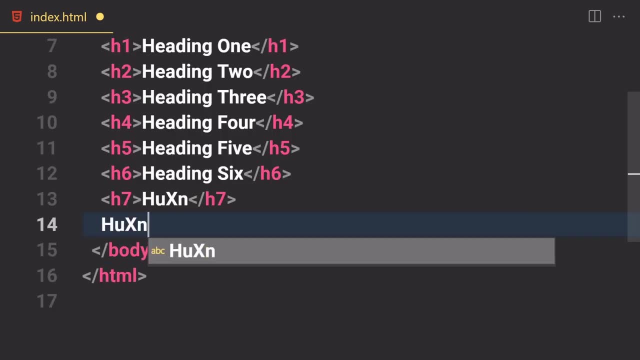 write h7 and if you just close that, and if i just type something like uh, i don't know, i'm going to just write my name like huzzain in here and you know what, and i'm going to just write huzzain without any code whatsoever. so now let's just see what will happen. so for that i'm going to just 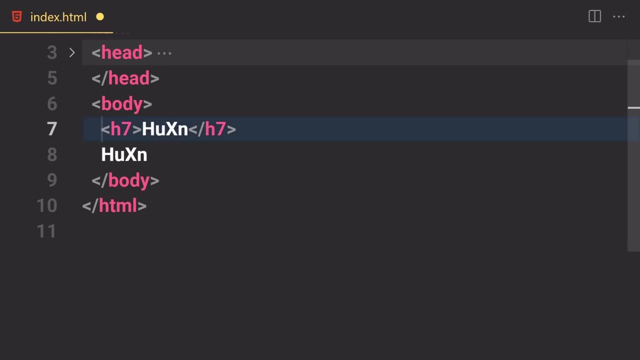 comment out all of this code, or you know, i'm going to just cut that for now and and now, if you save that. so here you can see we have, or h7, and we also have just a simple text right here. so now, if you sell that, 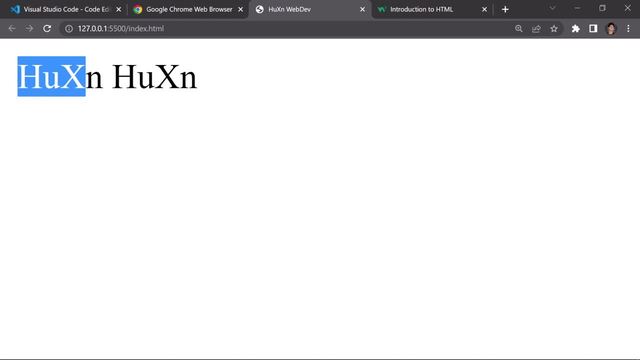 now here you can see, our browser will treat this at 7 just like no code word search. so if you just right click on that and then if we hover over to this inspect, and then we have to click on that, so it will now open us this uh, developer tools, which you are going to be learning a lot. 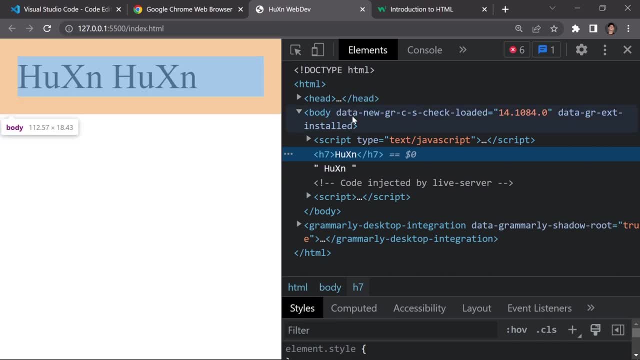 about these developer tools, but you don't have to worry about any of them for now. so what are we getting? we are getting, first of all, the dock type and, by the way, if it's by default like console, so you can just click on this element and i guess it will look like this in your machine. 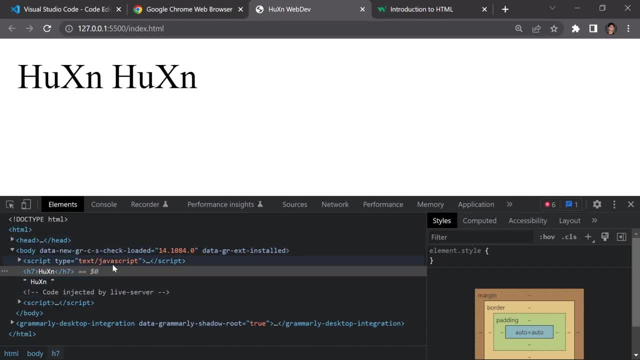 this is the first time you're opening there, so this is how it looks like. and now, if you want to take that like uh, to the left side or to the right side, so you can just click on that. and you can either click on this one and by default it will set like this one, and you can also just set that. 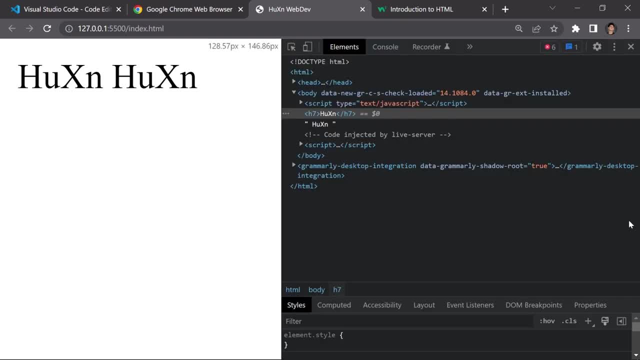 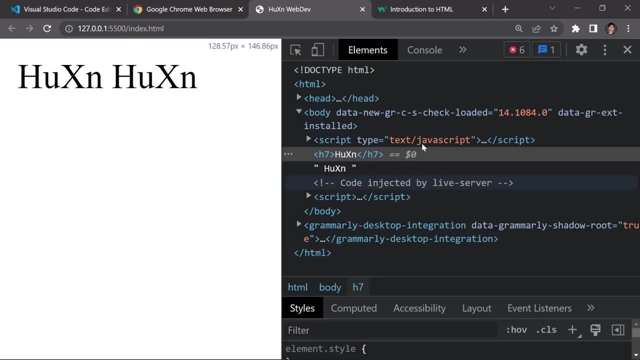 right here, like to the left or to the right. so if i just click on the right one and this is how it will look like. so if you want to zoom in, so i want you to just hold control and then the mouse in, like mouse scroll in and like zoom out, you get the idea. so here you can see, we have all of the html. 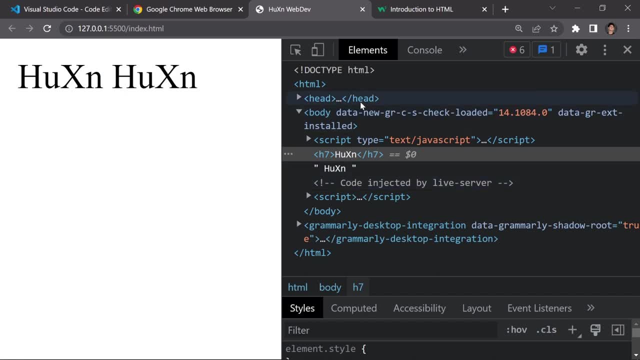 code, plus a little bit more stuff which you don't have to worry about it for now. so first of all we have this doc type html, as we learned that just a second ago. then we have our html opening tag, html closing tag, then we have our head area right here, so we have our title and then we have our script. 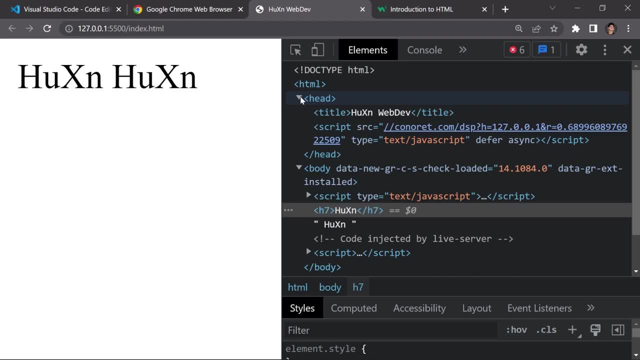 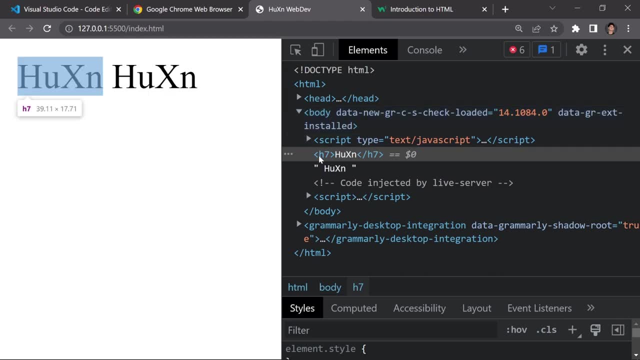 which is coming from a local server, which we've installed in our uh visual story recorder, which you don't have to worry about it for now. so i'm going to just collapse this one, then we have our body and then here you can see, we have this h7 right here. so i want you to just notice that. 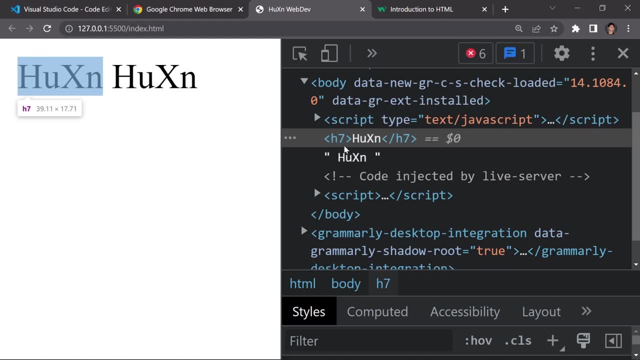 we do have this h7 right here, but our browser will treat it like a simple text right here. okay, so both of them are looking the same and both of them will have the font, so you don't have to worry about the font sizes and stuff right now, but both of them will just like. our browser will treat both. 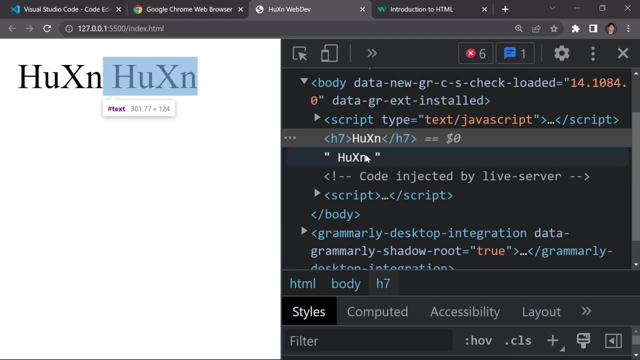 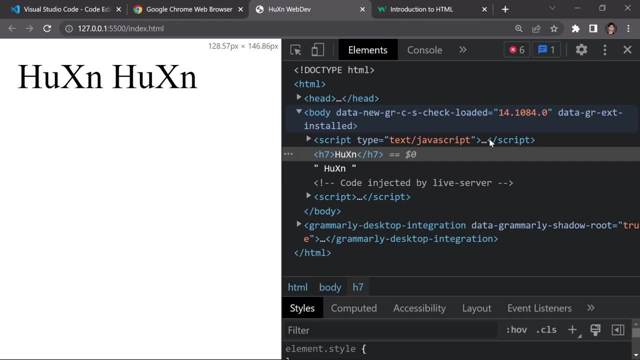 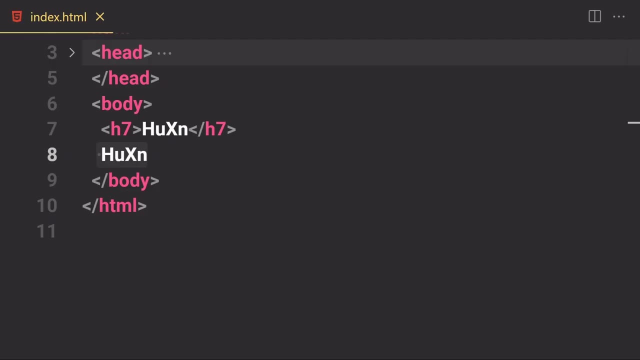 of them as just a simple text without any code, and we cannot select that once we jump into a css and we cannot do anything with that. so in html we have headings from h1 to h6, not more than that, or just cut this one for now and now. we have our screen right here and now. what do we have to do? 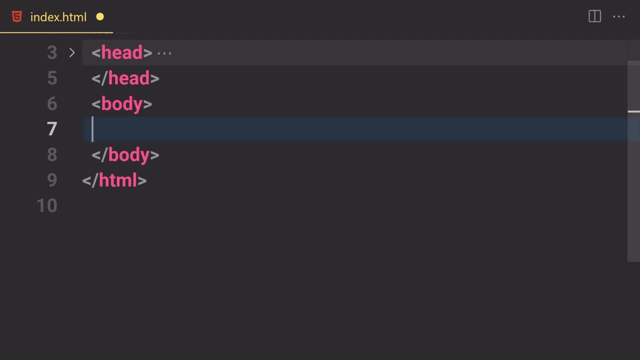 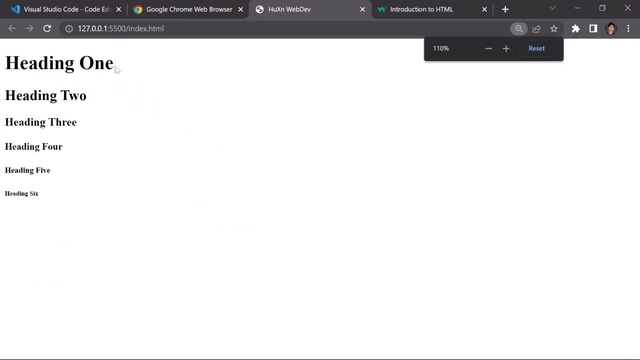 i'm going to remove all of that, and now i'm going to just hit ctrl v to paste all of my previous content which i just cut. and now, if you save that, and this is how our headings looks like by default, okay, so now we are totally done with the headings. so the next topic which i want to show you is: 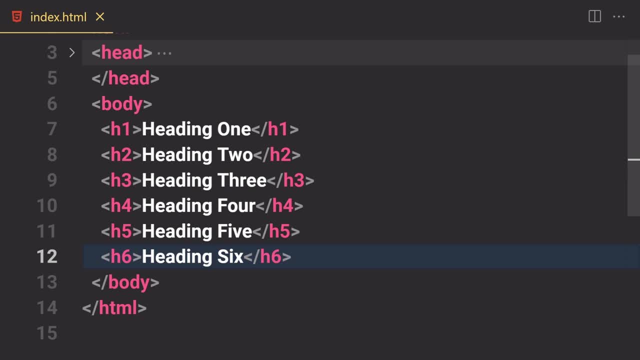 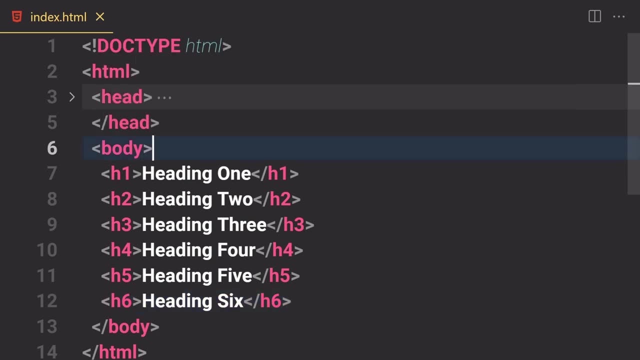 something called comments. so what are comments? as the beginning of this video i said like anything right inside a body tag will show up to the user, if except comments, and you may or might seen this one which i wrote in the beginning of the course, but i guess you didn't saw that. 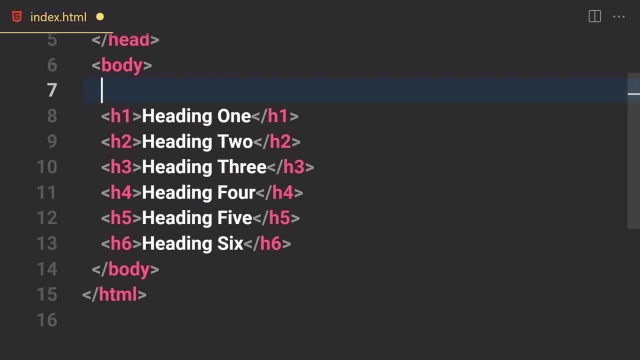 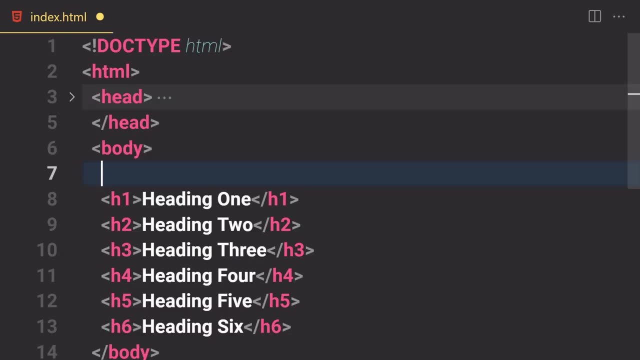 so now let me just talk about a comment. so a comments, as the name suggests, will be a comment for ourselves. so now let's suppose if you work on this file, like we just write our doc type html and stuff, and now that we know like what is the heading and h2 and h3 and so on and so forth, 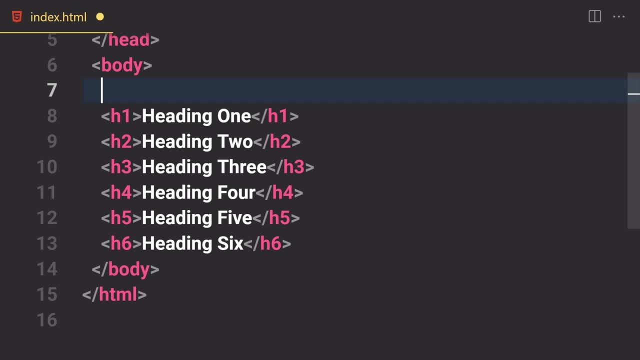 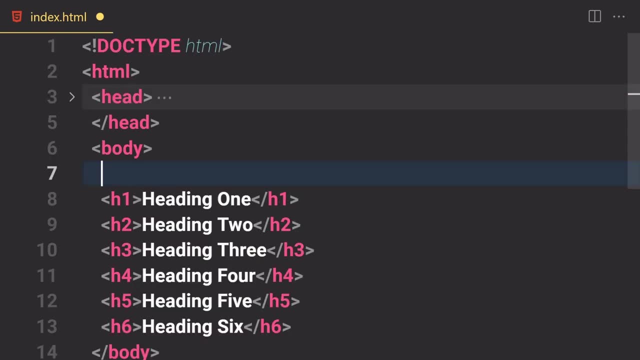 and now, if you want to write a comment for yourself or another note for yourself, so for that we are going to be writing or for that we are going to be need something called a comment. so later, like maybe a month later or maybe a week later, and if we open, 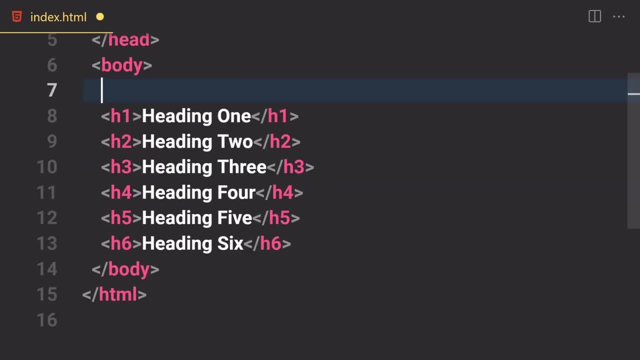 our file and we forgot like what is h1, h2 and h3 and so on and so forth. so we can also write or notes for us. so we can. if you want to write a note or a comment for yourself, so for that we have to. 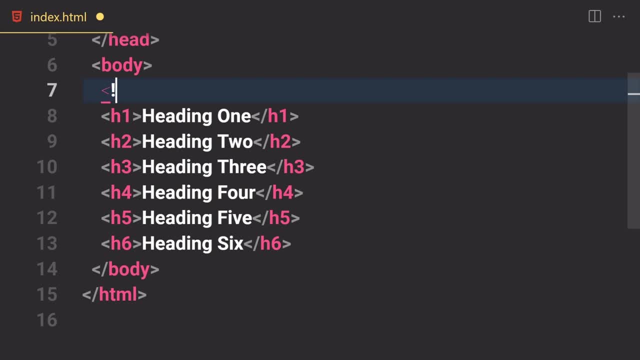 first of all write a less than sign and then this explanation mark, and then if we just write two dashes right here, so here you can see it on log uses these kind of syntax right here, so we have a comment opening and then we have a comment closing right here, so anything we write inside. 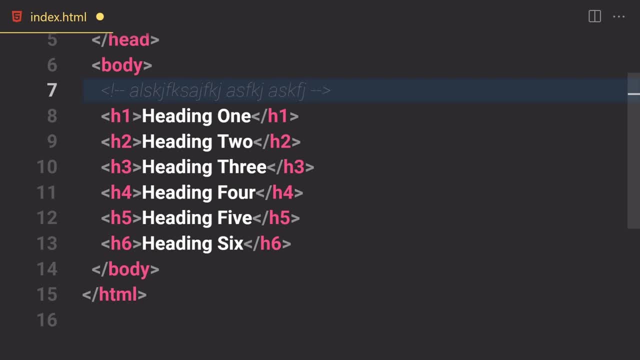 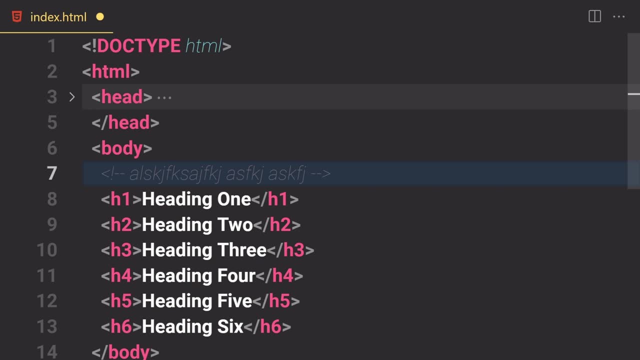 this comment will not show up to anyone because they will be ignored by our browser. so in programming in general, if you want to write a comment like, let's suppose, if you want to write a comment for in javascript file, so it will be ignored by a compiler, but now in this case, our 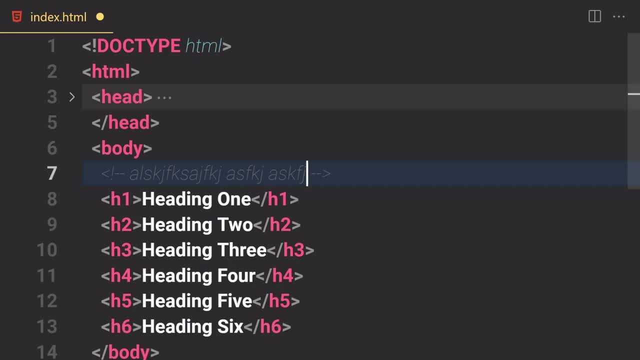 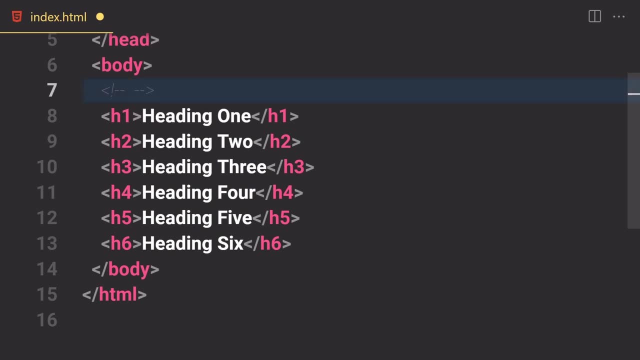 compiler is our web browser, so our comment will be ignored by our browser. okay, so we are going to. so, instead of writing all of these gibberish, so, i'm going to just write like, uh, maybe, uh, we've worked on headings, okay, and we have, like, you know what, we can also write multi-line comment, or we. 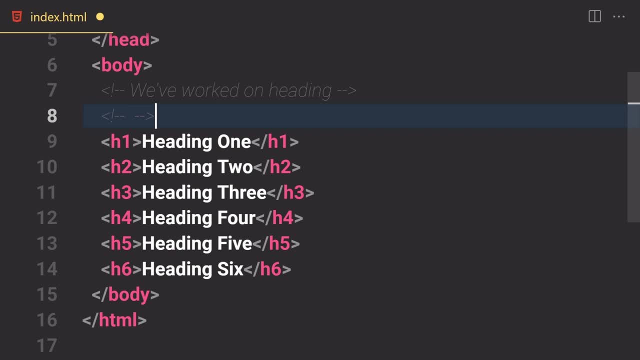 can also just write a new comment if you want to. and, by the way, the shortcut for creating a comment is that you just have to hold ctrl and then just hit slash, so it will not just create a new comment area for us. okay, and now let's suppose if you want to comment all of these area out, so for that we. 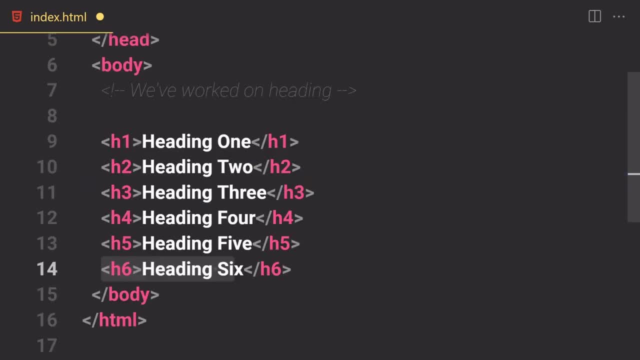 have the select these area or you know what. if you can just like select single item, okay, like we can also comment just a single element, or we can select all of them. so first of all we have to select some area or some specific code and then we have to just hold ctrl and if you hit, 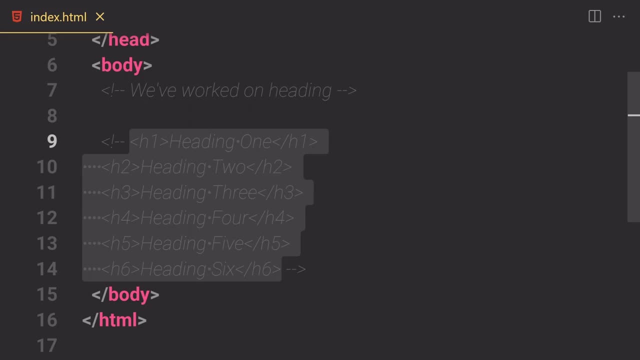 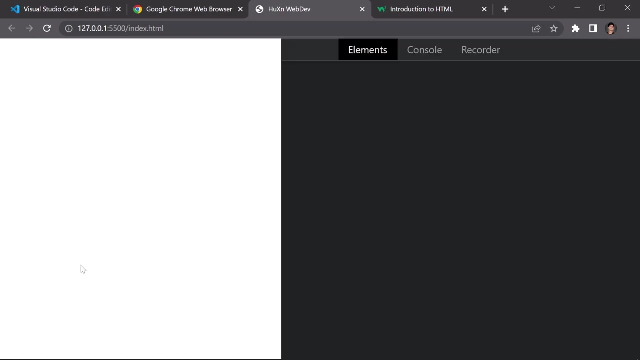 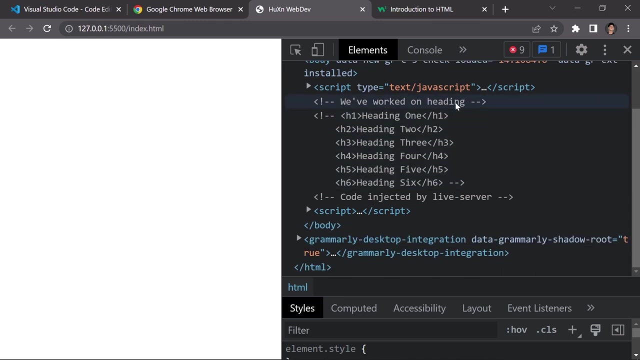 slash right here. so we will now just comment all of these codes. knife, you save our file and boom, everything is gone from here. but if you just right click on it and if you click on this inspect area and now if you just expand this body area or comments right here, like we've worked on headings and we have heading one, two, three, four, 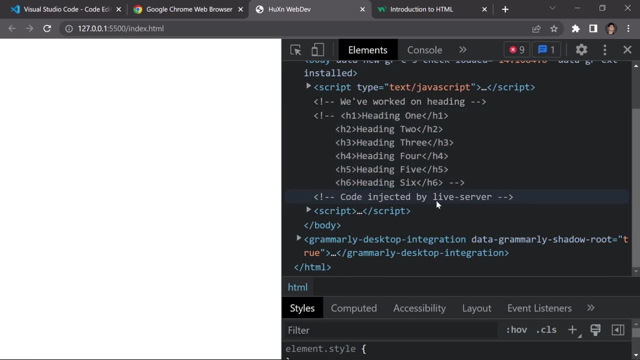 five and six right here and, by the way, you can also see this code injected by the live server and here you can see this comment is coming from a live server in which you don't have to worry because this is not our code and this is not our comment. okay, so comment can be helpful inside. 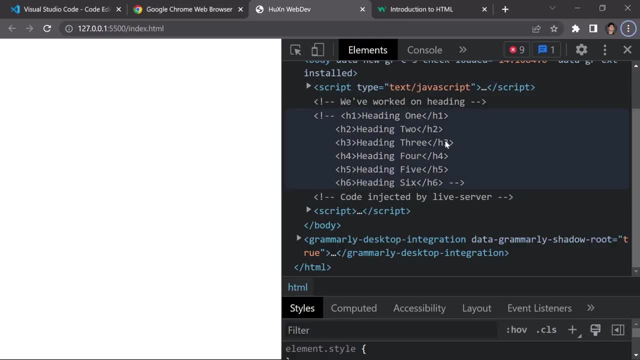 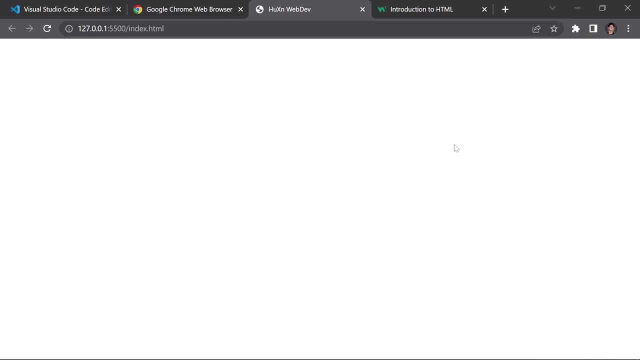 or coding, but not outside from a coding. okay, so i just kind of want to show you this um developer tools. so this is how you can find that. so i'm going to just click on this x and it will disappear. and now, if you want to uncomment this code, so first of all we have to select that. 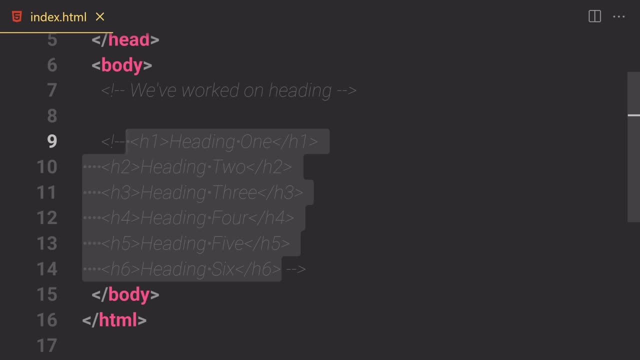 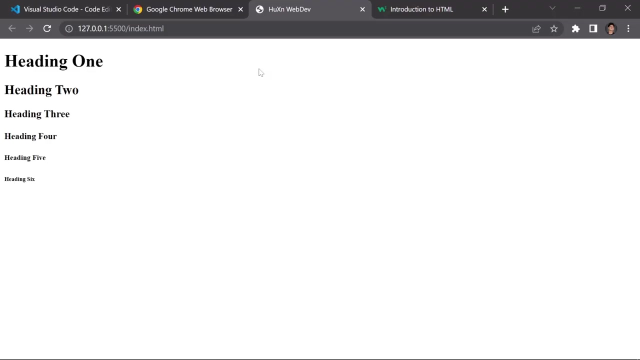 so now that we selected, and now we have to use that old command like control or command and then slash, so boom, it's now come up here again. and now, if you save our file and now here you can see, we have our coding back right here. okay, so now we just write this comment for ourselves. but we don't want. 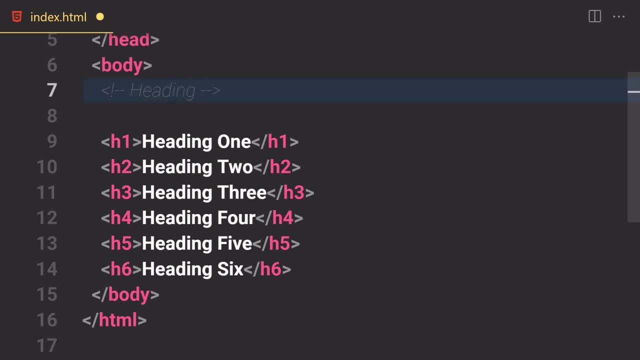 that. so we are going to be just writing like headings in this case, and now, if you save that? and then we are going to be just writing like headings in this case, and now, if you save that, nothing will happen, as you saw just a second ago. now, the next topic which you are going to be: 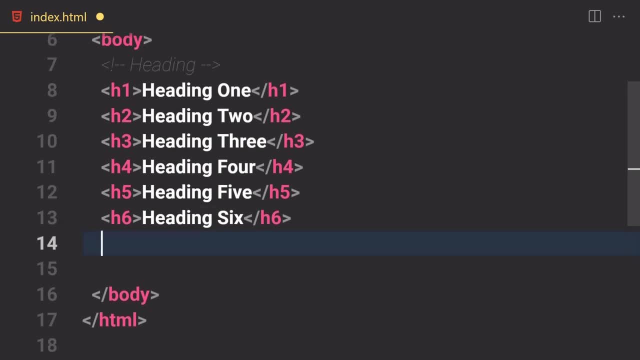 learning about in this section is something called paragraph. so we don't have to write a comment for every line of code we write, but we can just write a notes for itself, you know. so if you want to provide a note, so in this case i'm going to just write like para graph right here. so now, if you, 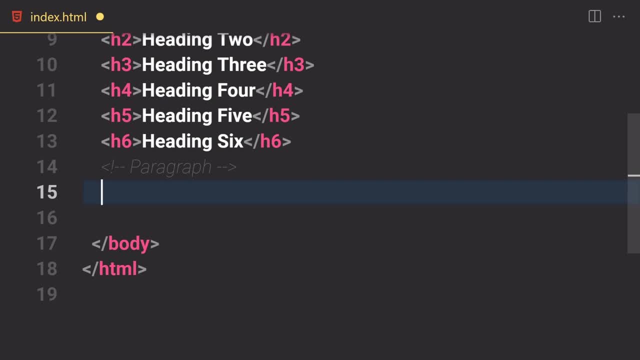 are working on a paragraph. so what do we have to do? we just have to write p and if you hit tab, server log uses paragraph opening tag and paragraph closing tag, and anything we're writing inside this p tag will be or paragraph, as the name suggests. so i'm going to just remove. 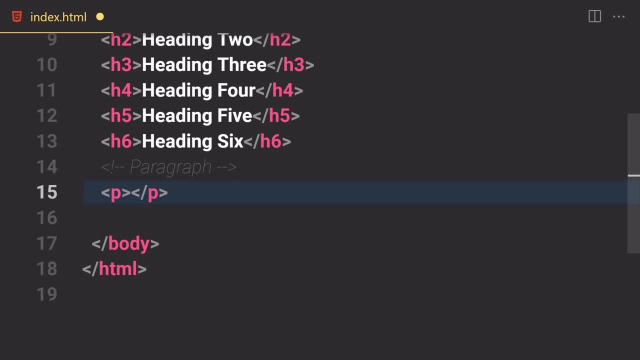 this gibberish from here and i'm going to just put my uh own name right here, like huzzain maybe, or huzzain webdev, or you can just type whatever you want, okay, so in my case i'm going to just stick to huzzain webdev. and now, if you save our file and here you can see, we are now getting these. 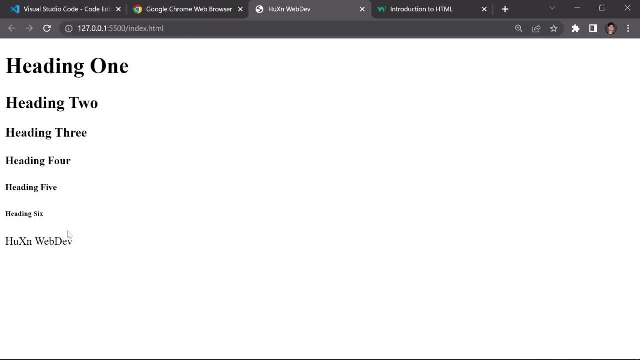 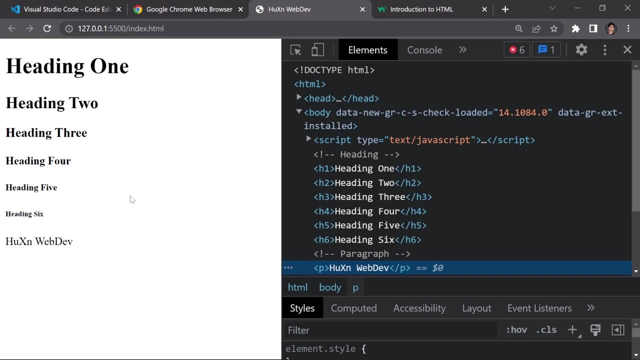 huzzain webdev right here. so if you just right click on that and if you click on this inspect- and, by the way, if you want to get this inspect area without clicking on a specific elements, you can just hit that ff l, so we'll now just close it. and if you hit f12 one more time, so it will now open it right here. 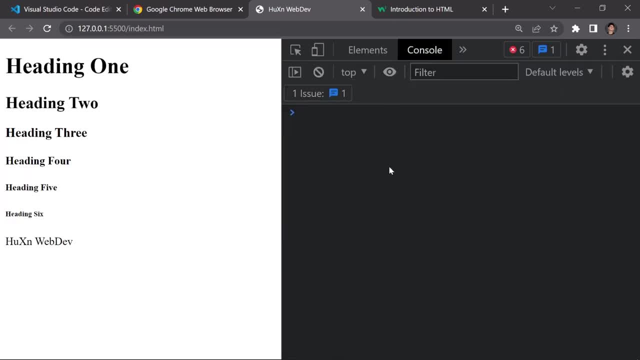 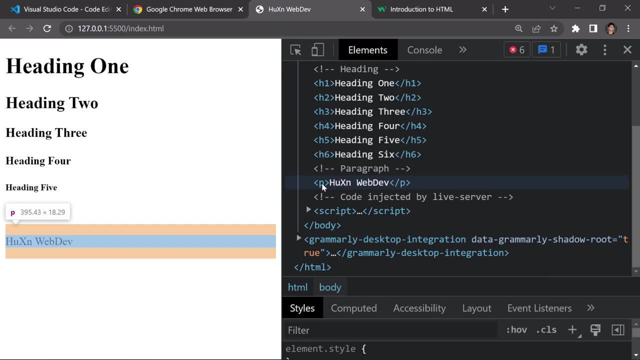 okay, and i guess by default it will just open the console area and you can just click on then the elements tab. so it will now just open the elements tab for us. and now here you can see, we have this paragraph opening tag and paragraph closing tag, and then we have our content inside this paragraph. 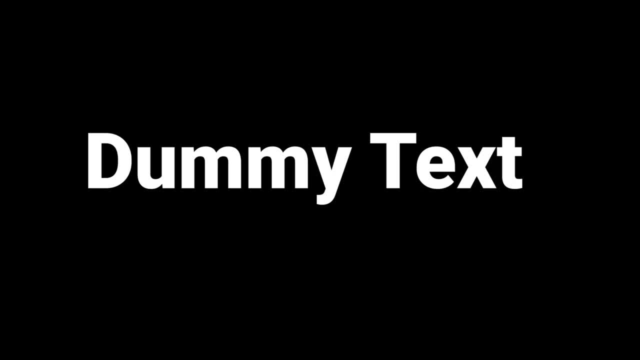 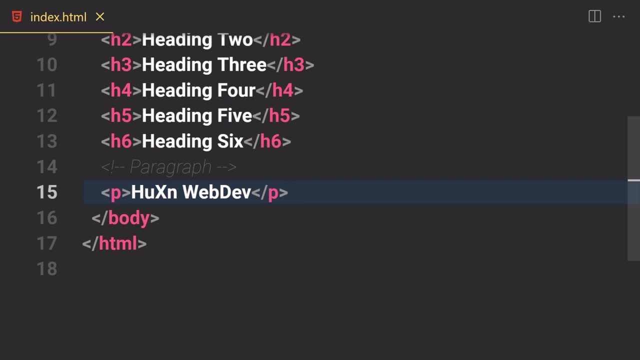 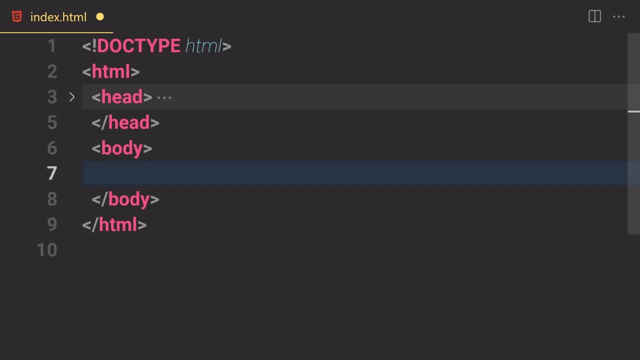 okay, so these are the headings and paragraph in html. the next topic which i want to show you is something called lorem ipsum. so you know what? first of all, i'm going to just clear out my body so that we can work on a lorem ipsum. here you can see, we just have our structure and 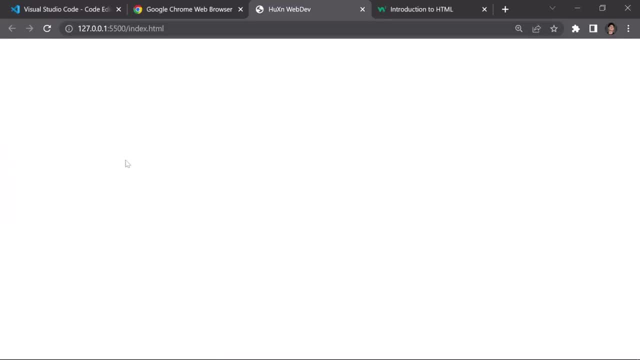 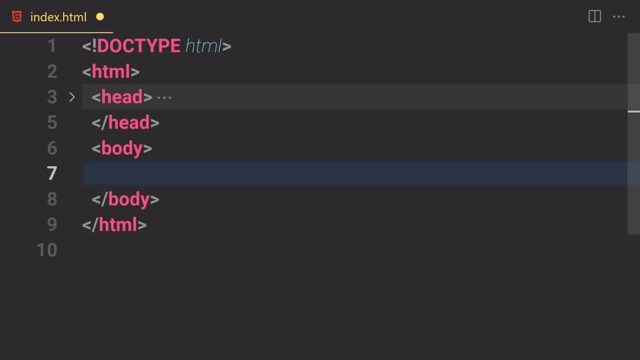 then we have our empty body. so if we save that and nothing will show up right here because we don't have any content inside this body area. so now if you want to work with a lorem ipsum, so in some cases you would need a lot of text in your project. like like a lot of text, like just random. 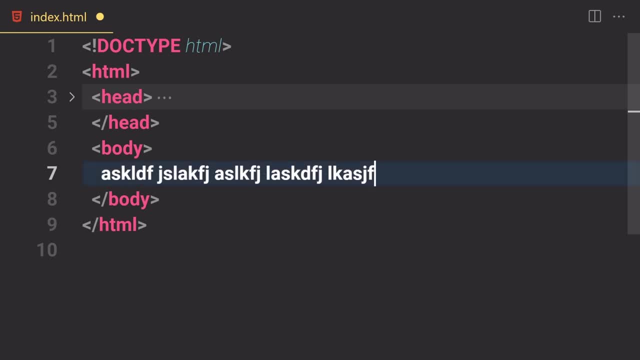 text. so you cannot write random text like that. it will look really messy and really ugly for other engineers and also for yourself. like you cannot write that you can, like you totally can, but it will look ugly. so if you just write, you know i'm going to cut all of these. 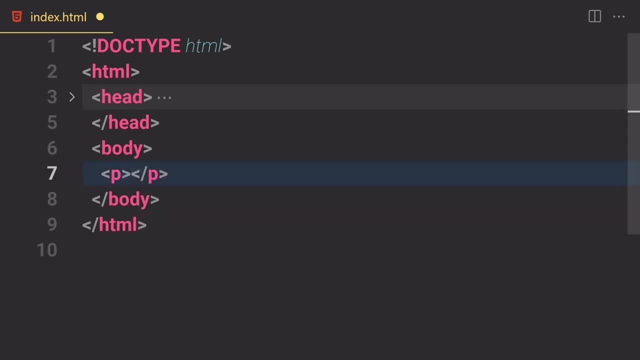 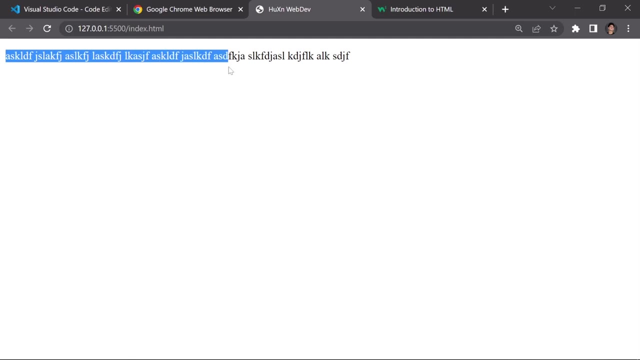 gibberish from here and i'm going to just write p and inside this p i'm going to paste all of my text by pressing ctrl or command v. so now, if you save that and here you can see, we are now getting this gibberish. but you can also notice like: first of all, it took a lot of time to write, so we just 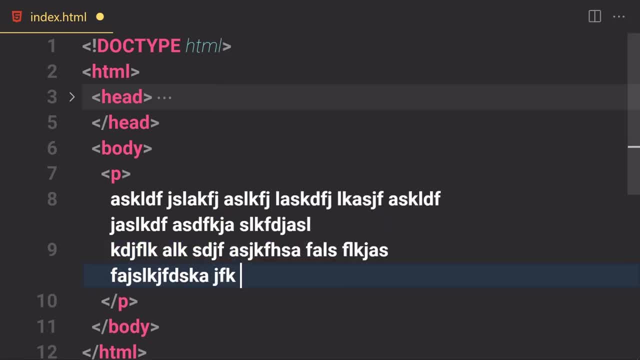 have to write like all of these random uh words right here and now the next thing we have, like it looks a little bit messy and totally ugly, okay, so unreadable if you save this more text. so here you can see, uh, they are looking totally ugly. so now, in this case, we are going to be removing all. 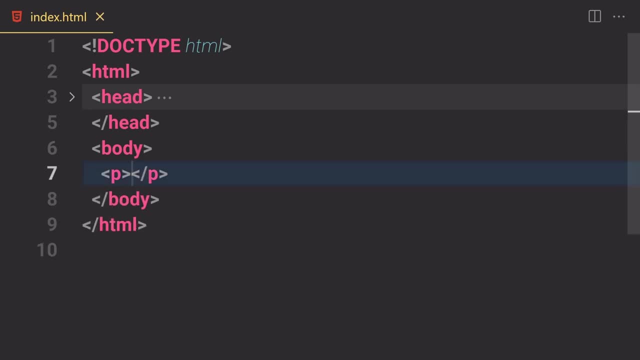 of these texts from here and instead we are going to be writing something called lorem ipsum. a lorem ipsum is nothing more but just a dummy text and i can just guarantee for a visual story coder and i cannot guarantee for other coder out there like jet blinds or adam or stuff like that. 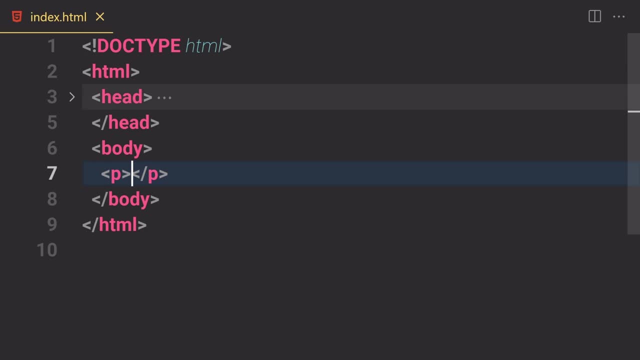 sublime text. i cannot guarantee for that. but in visual story coder, if you want to generate a lot of text like a lorem ipsum, so for that we can just first of all write a lorem keyword and then we can specify the amount of words we need. okay, so if you just click on this image, abbreviation, so here you. 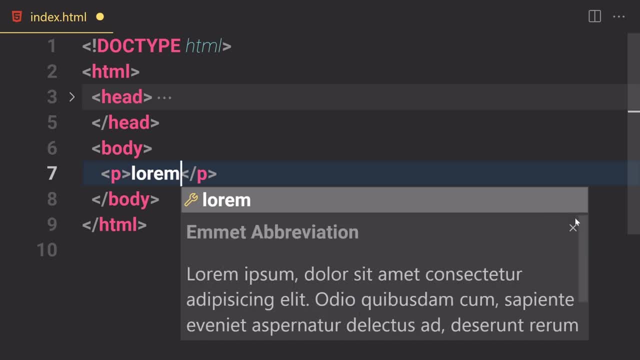 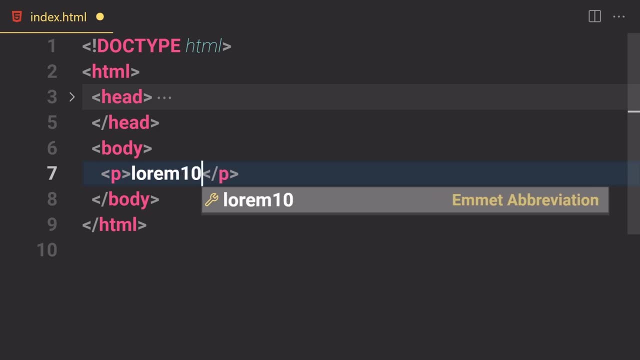 can see. it now just gives us all of these random words right here. so you know what i'm going to just put like maybe 20 words, or you know what i'm going to put like 10 words for now, and if i hit tab, so here you can see, the log uses like 10 words and if you see 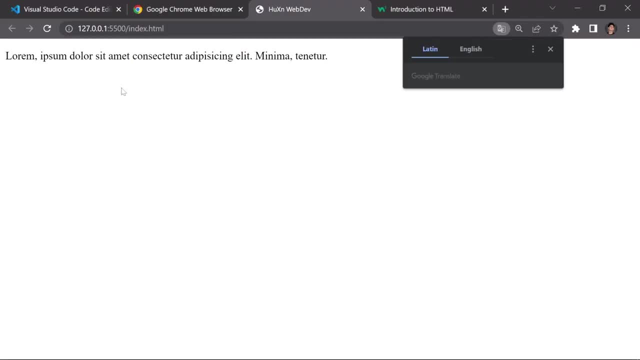 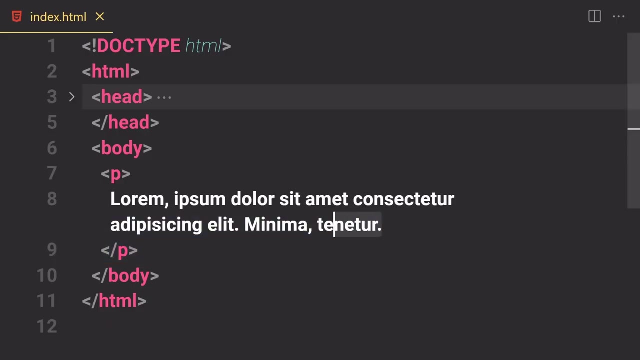 save that and boom, it will log. uses a 10 words right here and my browser will by default detect like latin words, and i guess it's not a latin. it doesn't even mean anything, like we have lorem ipsum, dollar, seed amid and stuff like that. i can't even pronounce other words anyways, so let's suppose so. 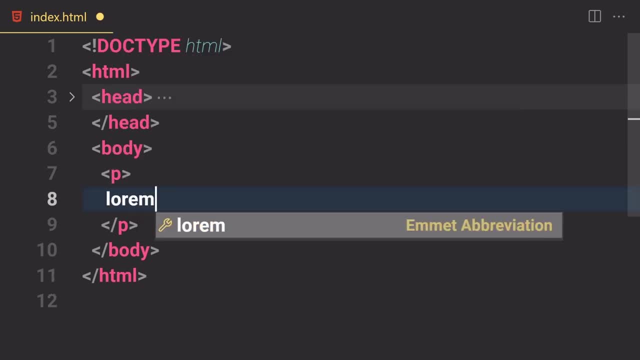 that was just- uh, i guess, 10 words i just wrote. we can also write like a: first of all just write a lorem keyword, and then we can specify like maybe 100 words, so i'm going to just write 100 and then. so here you can see, it'll now just generate a hundred words for me. so now, if you save our file, 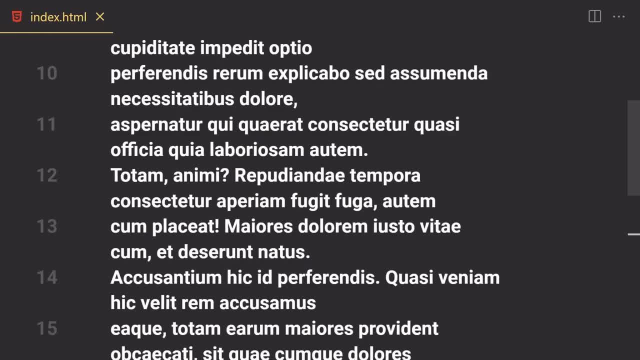 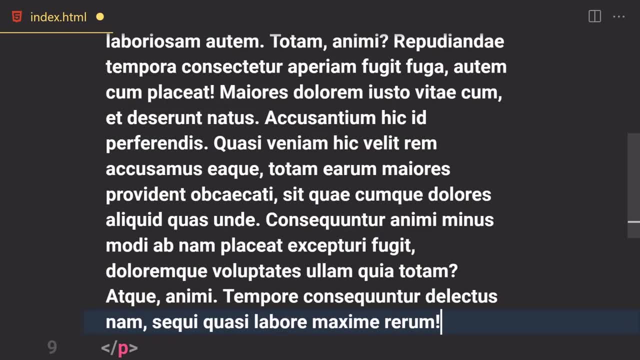 and here you can see we are now getting 100 words right here. okay, and now, if i want to undo these steps, so we have to just hold ctrl, and if you hit z, so we'll just undo it one more time. so now we have to do that one more time by holding ctrl and hitting z, so it will just undo that step for us. 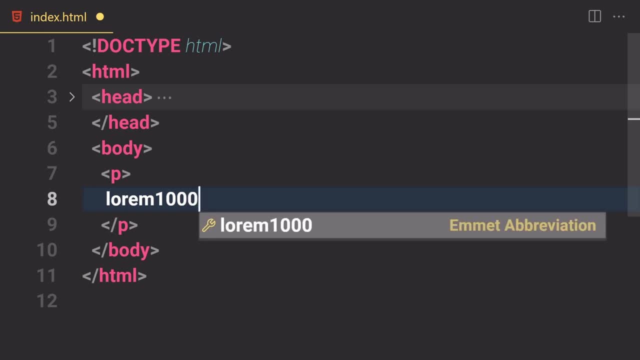 and we can just write like maybe thousand words, if you want to. in some situation we would need like a thousand words. uh, i guess that that situation won't come, so i'm gonna just write, i'm gonna hit tab right now and it will log users: thousand words, right. 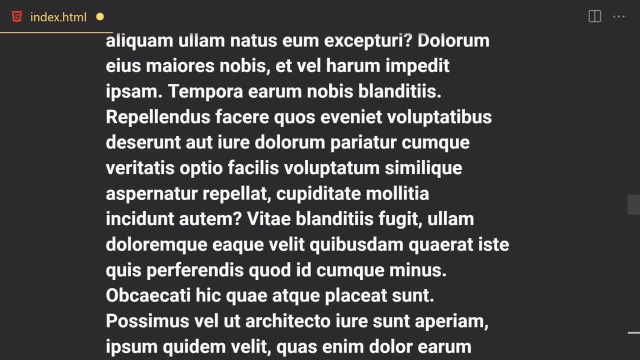 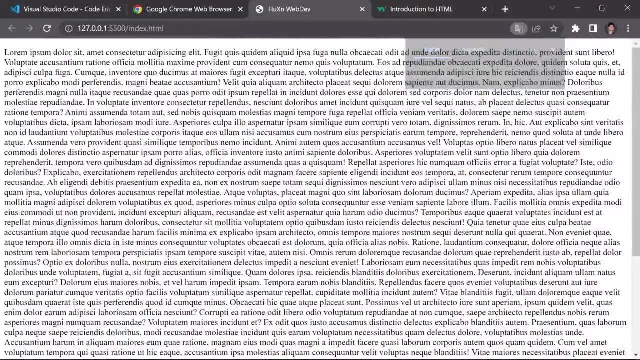 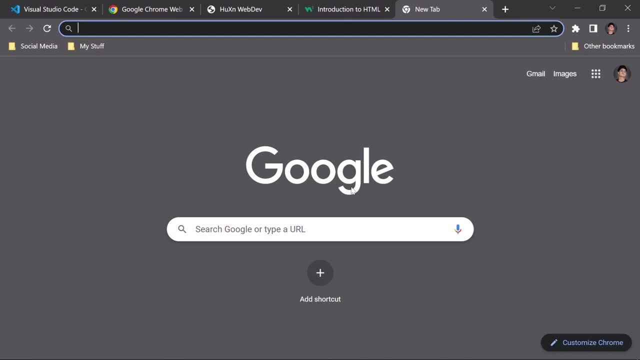 here. so now, if i just save my file by holding ctrl and hitting s, and boom, it will log you this thousand words right here, a lot of lorem ipsum. and, by the way, if you want to check out the lorem ipsum website, so you can just go to your google and here you just have to type like um lorem ipsum. 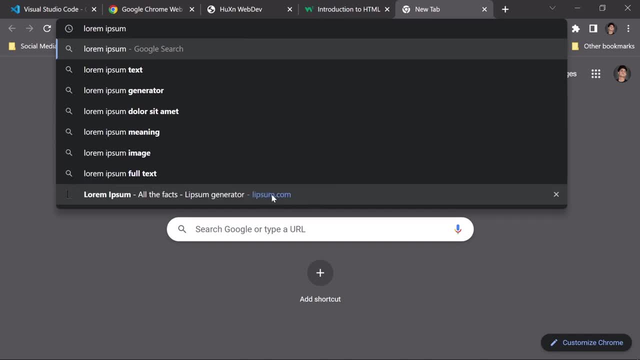 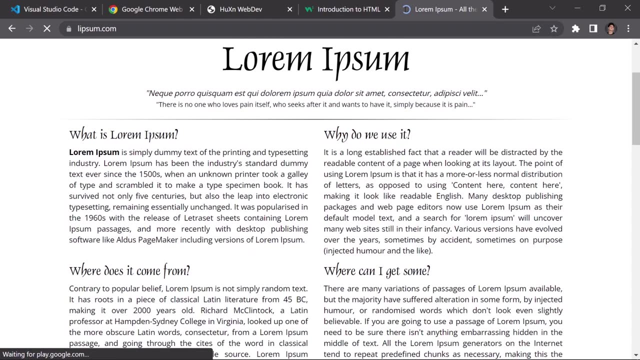 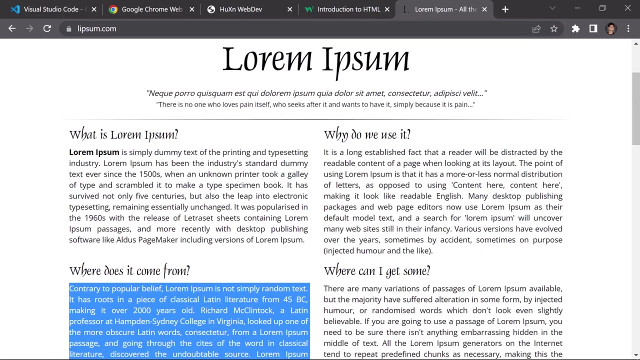 okay, so here's the website which is known as this lipsumcom, so you can just click on there. have just lipsumcom. it will now bring you to this page. right here you can learn more about lorem ipsum, or you can also copy- uh, these actual text if you want to. so lorem ipsum is simply a demo text and 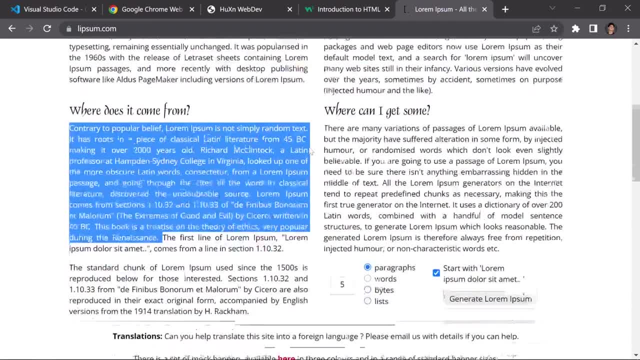 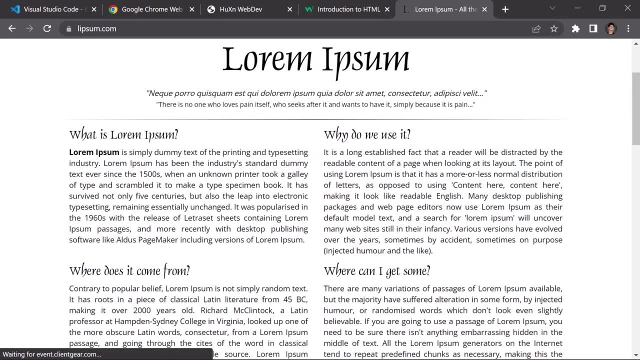 blah, blah blah. you can learn more about, but my suggestion: do not waste your time on learning about lorem ipsum. you just have to remember this one line like lorem ipsum is simply a dummy text, okay. so if you need some dummy text over there, you can just write a lorem keyword and you know what. 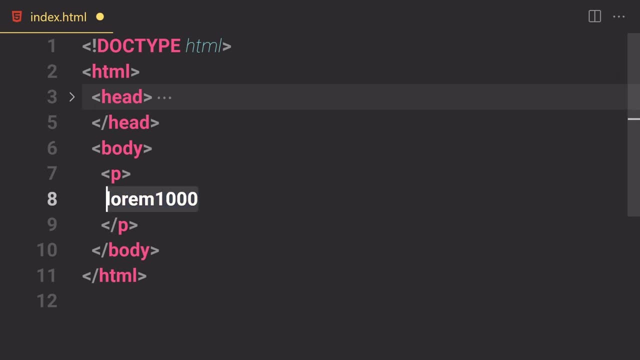 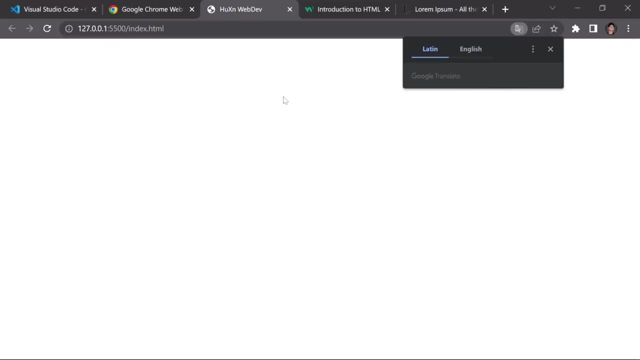 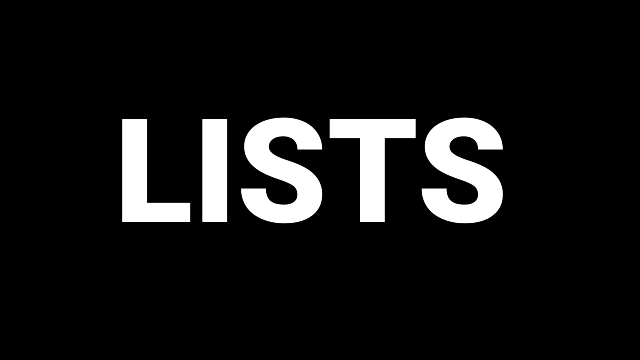 will see one more time and it will now just undo that step for us. so that was it about for lorem ipsum. i'm going to remove that and save our file and boom, we don't have any content whatsoever inside this page right here. okay, so that was just kind of it about for lorem, if some paragraph and headings. now the next topic. 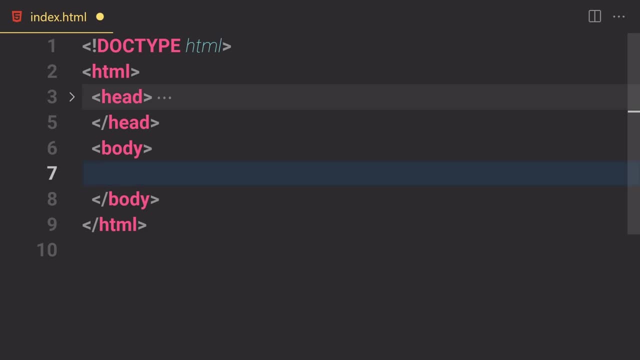 which you are going to be discussing is something called lists in html. in some situation, you would need your data to be in order, and in some situation you would need your data to be in order, like, let's suppose, if you are building some sort of application for maybe a lot of fruits. so 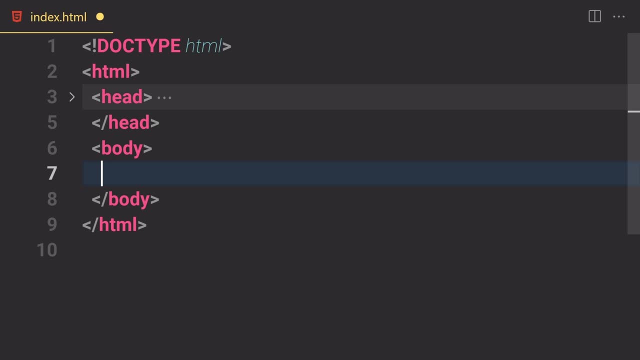 you would need your fruits to be in order like one, two, three, four, five, six and thousand and stuff like that. but in some situation you would need just a bullet points like bullet one, bullet two and stuff like that. so for that we can use a list in html. so how can we go about doing that? 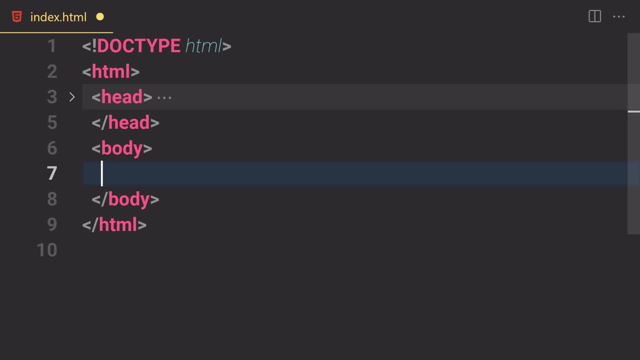 so in this section we are going to be learning about three kinds of in HTML, And I guess you can also find like more than three ways to write your lists. But I will not suggest to waste your time on list because you will need a list, just in a very real tiny. 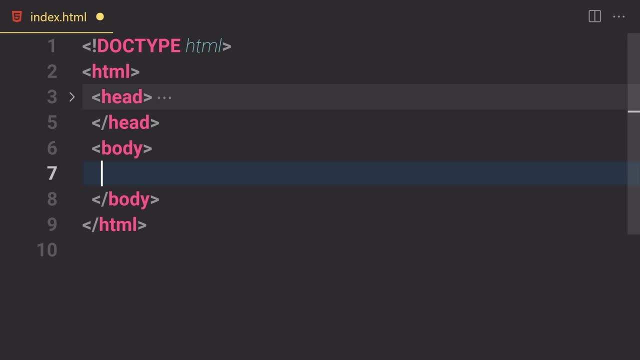 scenarios, but not in a lot of cases. Okay, so we are going to be just writing, first of all, the order list, and then we are going to be writing an order on or dirt list, And then third list, which you're going to be learning is something called nested, and then list. Okay, 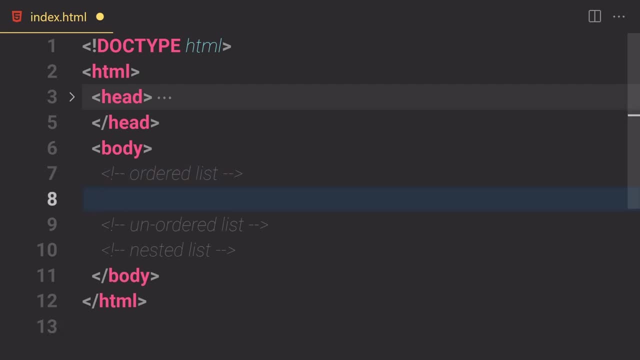 so we are going to be starting from the first one, which is an order list. So anytime you want your data to be in order, So for that we just have to write like O, L, And if you hit tab, so here you. 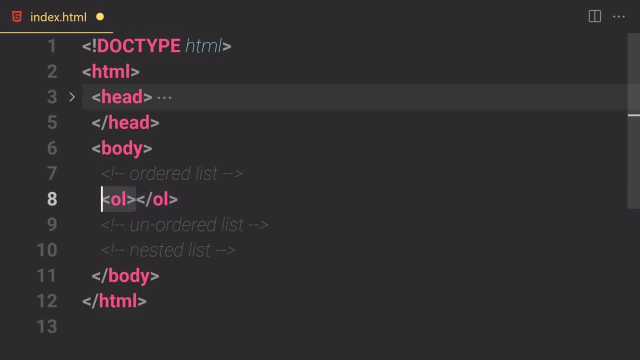 can see the log users: like order opening tag, like oil opening tag and then oil closing tag, And this oil just stand for like or list like order and list like O L. Okay, so now inside this O L, we are going to be starting from the first one, which is an order list. So for that we just have 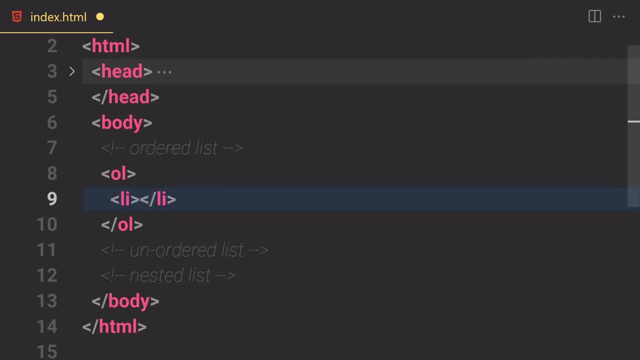 to write like O L And if you hit tab certain log users, like O L opening tag and then O L closing tag And this L I just stand for like list item. like L I list item. Okay, So here you can just put. 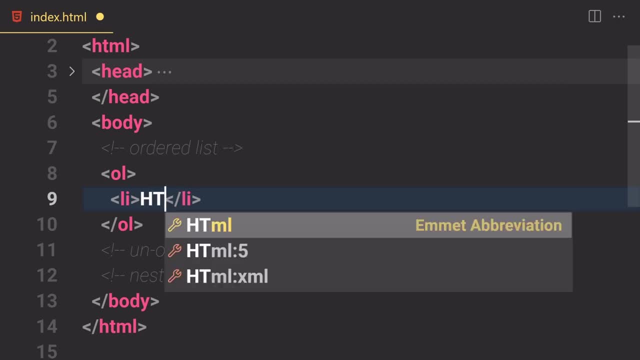 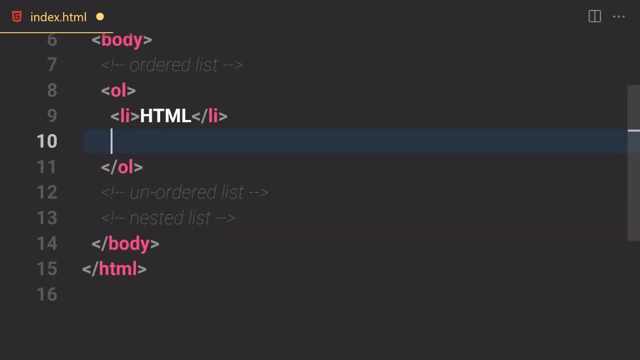 your data. if you want to like, in my case, I'm going to just put a technologies HTML. then we can just write like countless allies inside this oil, Like it doesn't matter, like if you write 10, 20100, 200 like 200 or stuff like that. we can go crazier if you want to, but in this case we are going to. 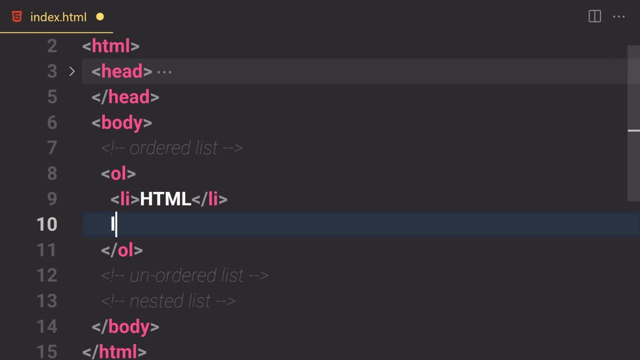 be just writing like maybe three of them or maybe four of them. i'm going to just write like li one more time, and here i'm going to just put like css. so in this case we just write like first html and then css. so now let me just save that file so that you guys can see what i'm talking about. 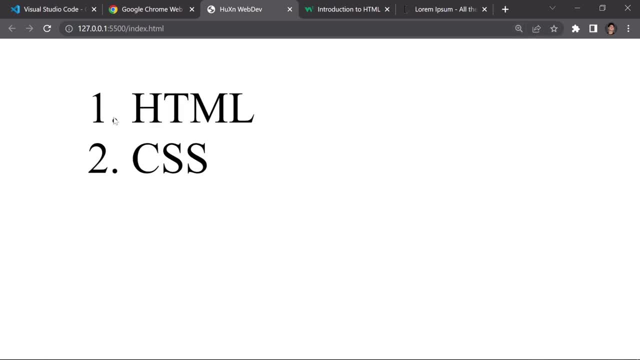 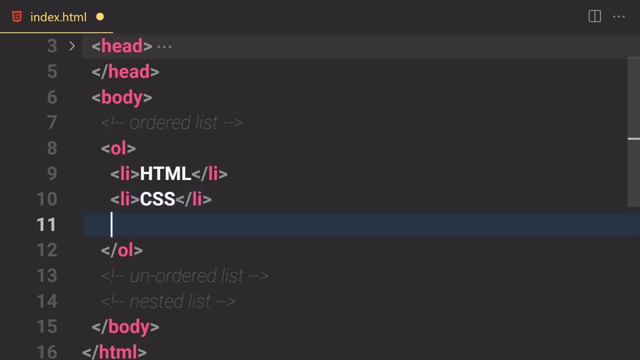 and now, here you can see the log users: one period, or dot, whatever you want to call it, and then we have our html, then we have second, and then we have a css, and this list can go on, and on, and on and on. so you can write like as many list item as you want. so i'm going to just write like li one. 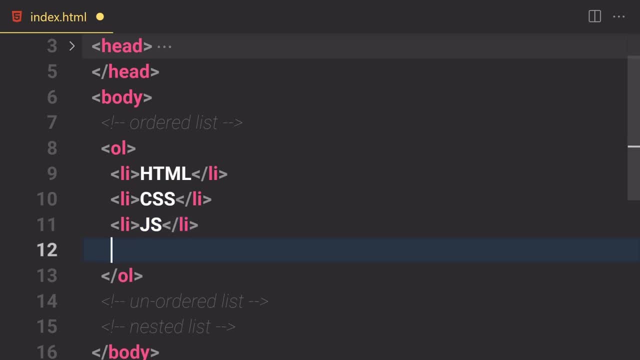 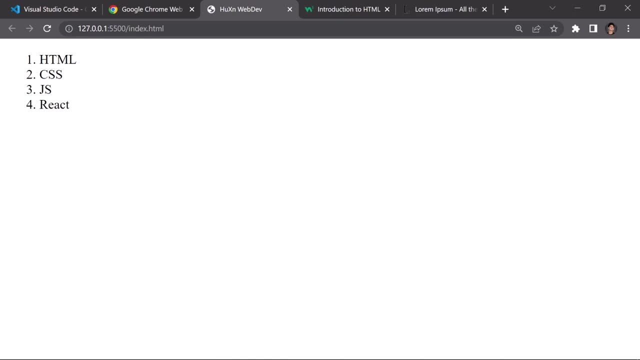 more time, and here we are going to be just writing, like j s for javascript, li for react, and this list can go on and on. so if you save that, and then it will give us like uh, one html, two css, three javascript and fourth, react. okay, so this is it about. 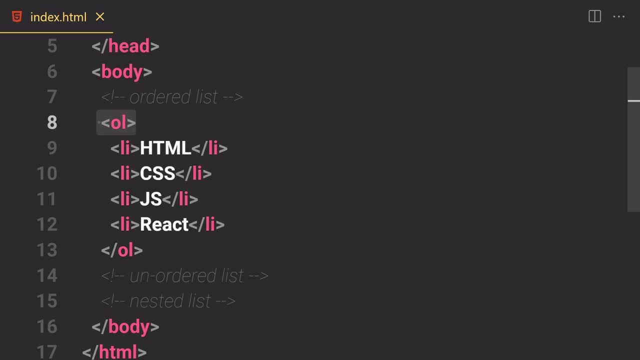 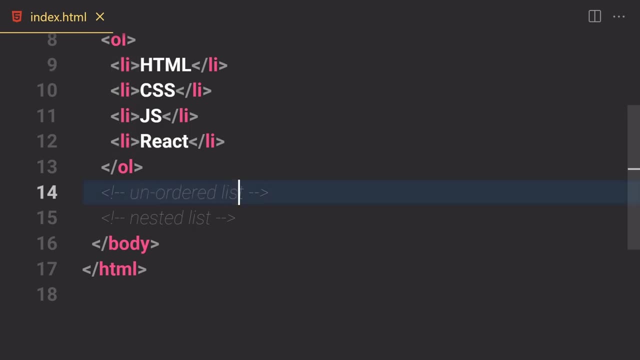 agency: six five, six, seven six five. so that's our list. so let me go ahead and see what we have- a ol like order list- and then inside this order list we are going to be writing or li for a list item. okay, so now let's just learn about something called unordered list in html. okay, so in some 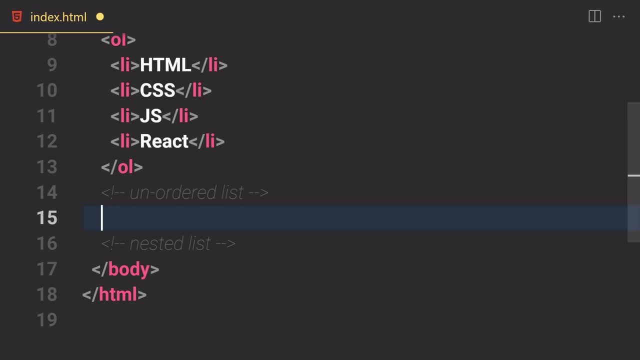 situation we would just need like a bullet points we don't care about like a main list. so for that kind of situation we can use an unordered list. so anytime you want to work with an unordered list, so for that we just have to write like ul and ul just stand for like unordered list. okay, so if you 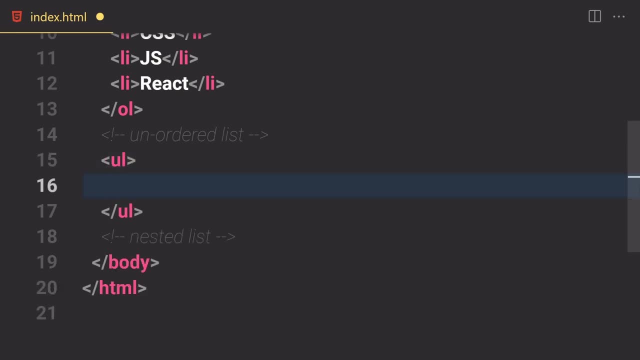 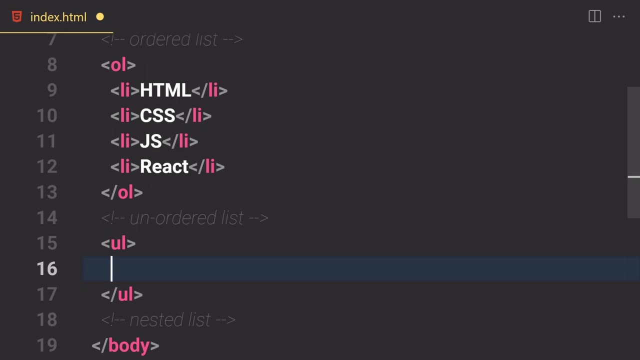 hit tab and now inside this url, what do we have to do? we have to just write: or li opening tag and li closing tag, and what is the li mean? i'm just asking you a question like: what is the li mean? i just i just told you a second ago, so i want you to tell me, like: what is the li mean? i'm waiting. 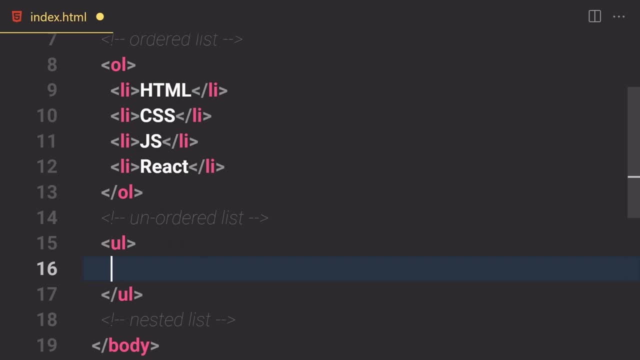 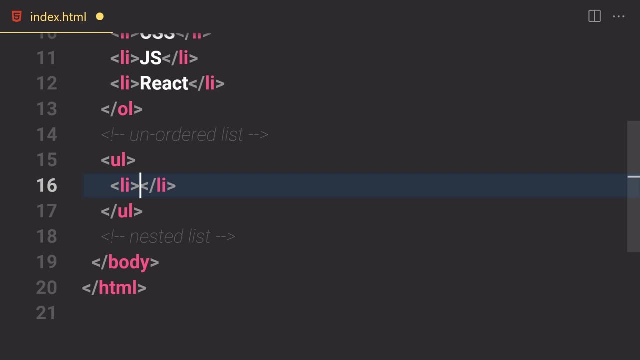 i'm just kidding, like li just simply means list item. so here we just have to write li. and if we hit tab and now here we can just write like uh, maybe a random people name someone, or just write like a peter, and then i'm gonna write one more li and i'm gonna write like john, then write a line of john, doe, let me. 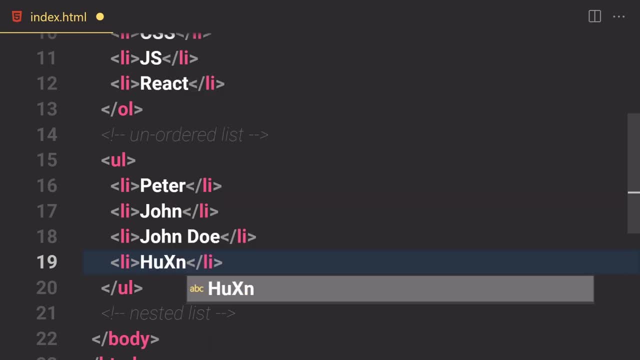 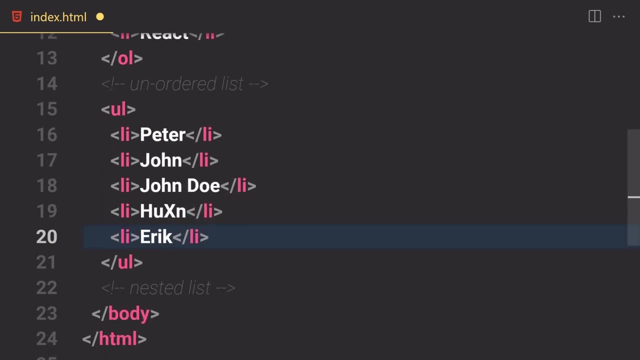 just write like another li of my own name, like huzzain. now let me just create another one, so it will be maybe eric, so i guess that would be fine for now. so if you sell file and boom. so here you can see, this one will be order list and this one will be unordered list. so here you can see we are. 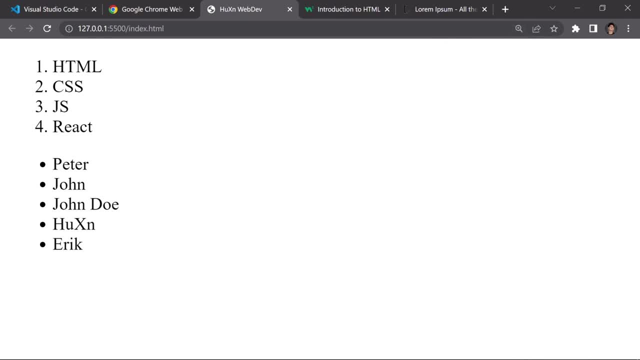 getting these bullet points right here. so anytime we just write a new list item and it will give us these bullet points right here. okay, so this is it about our order list and unordered list. so now the next topic which you are going to be learning is something called a nested list. so what is a nested 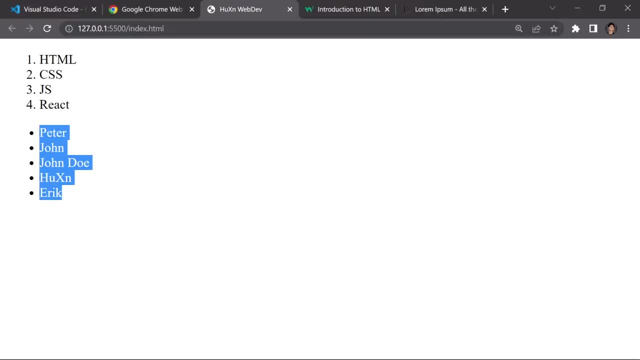 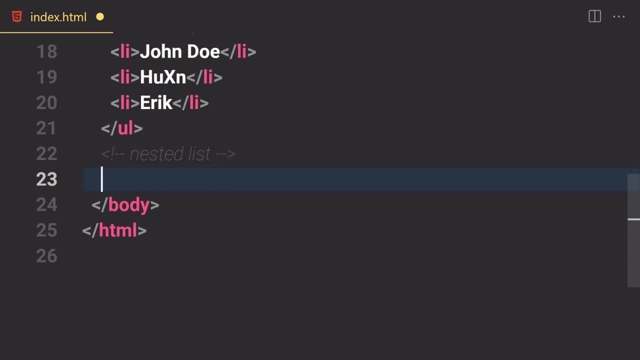 list even mean a nested list is a list inside another list. i know i'm just talking like a crazy person, so let me just write some code, then you will get to know what i'm talking about. so a nested list is a list inside another list, so that is known as a nested list. so first of all we have a ol like: 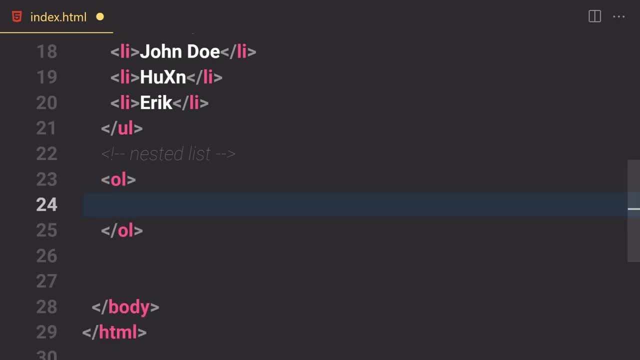 tag and ol closing tag. and now inside this oil we are going to be writing or li for a list item. and now here we are going to be just writing, or itself, like let me just write like my own self, like huzzain, and huzzain know these kind of technologies. so now here, this is a parent uh list, right here. so now. 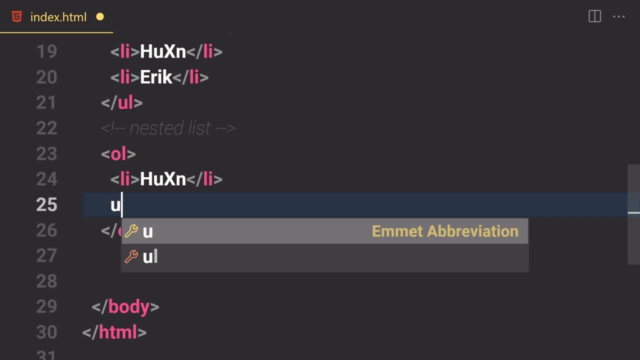 inside that we are going to be creating a new list, so i'm going to just write like ul and if i hit tab right here and now inside there we are going to be just writing li right here. i know these are different elements, so it's a little bit different, but you don't have to go that much. 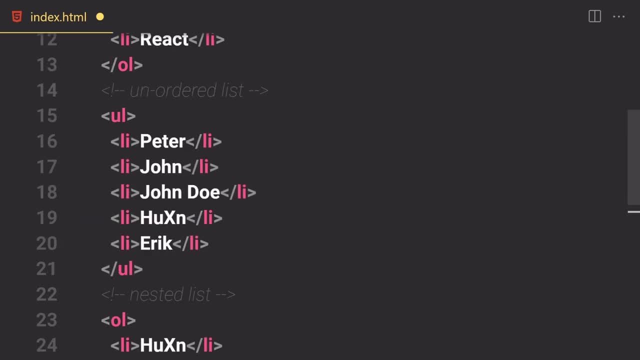 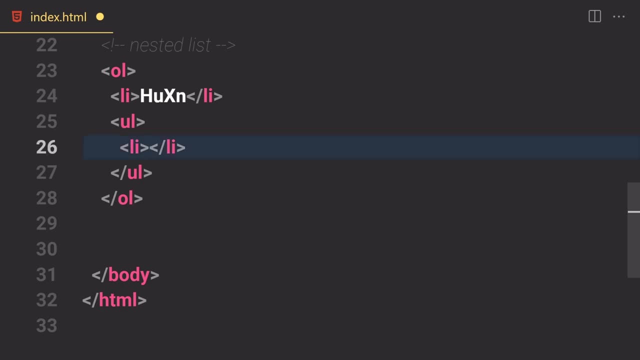 crazy. i'm just showing that for those people who are interested in a lot of lists. but you don't have to go like that much crazy. if you don't want to, you can just work with a ul and oil if you want to. so i'm just showing you for those people who are interested in these ul or nested tags and 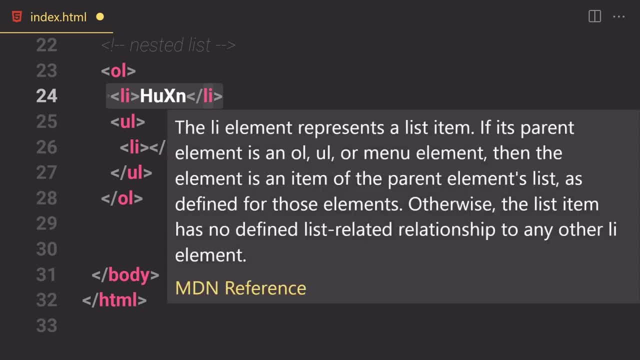 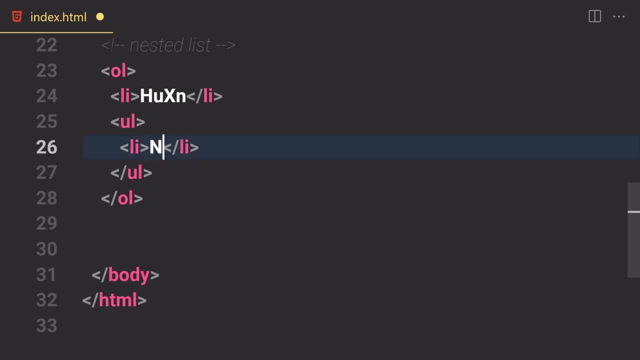 stuff like that. so first of all we have our ol tag, like oil opening tag and oil closing tag, then we have just one single item inside there and then we have another like hosanna, like nodejs. you can put whichever kind of text you like. and let me just create a. 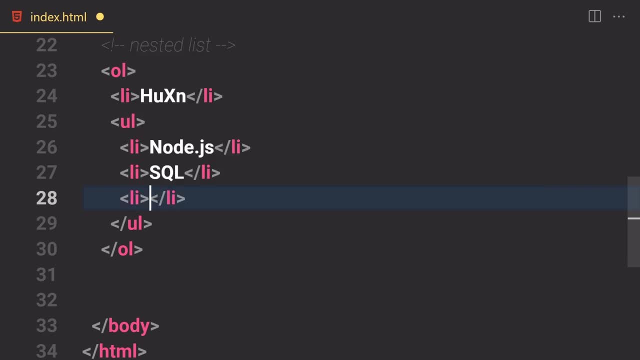 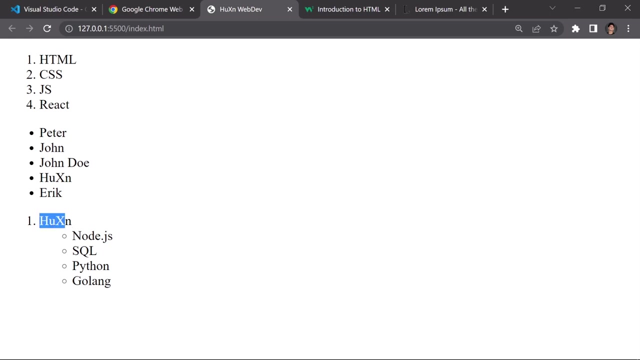 new li like sql for structured query language, li for python and also li for my favorite programming languages as a goal link. so i'm going to just save my file. and now here you can say: this is what a nested list looks like. first of all, we have a one list, then we have another list inside. 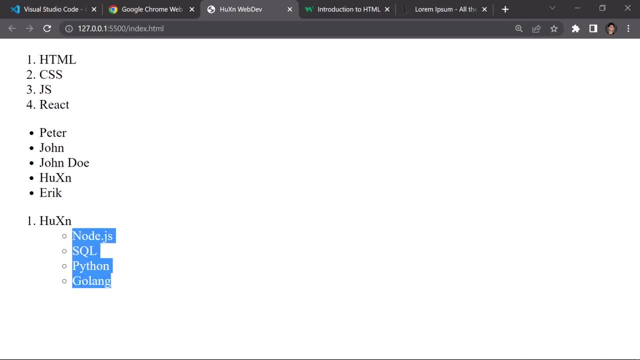 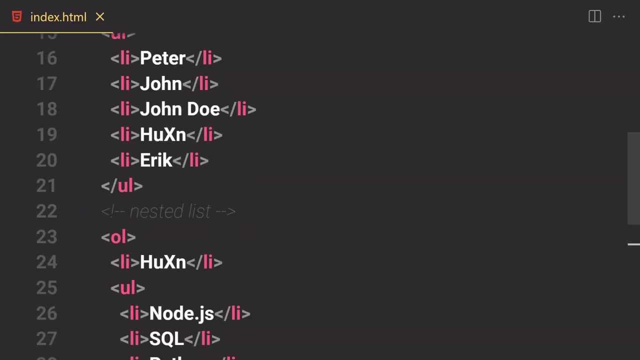 that list. so this is known as a nested list. okay, so now let me just zoom in a bit so you guys can see everything a bit better. okay, so this is the first list, like a parent list, and this is the children of this parent list. okay, so now we are getting this nested list, all right. so that was it. 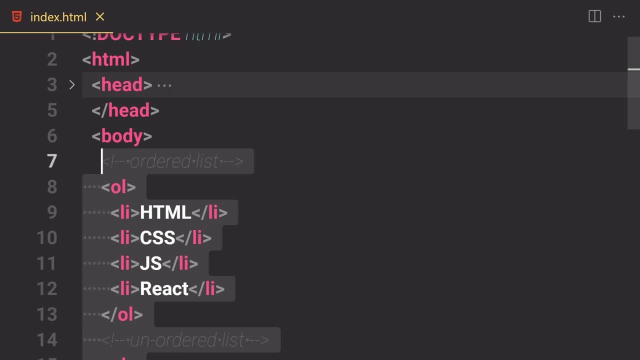 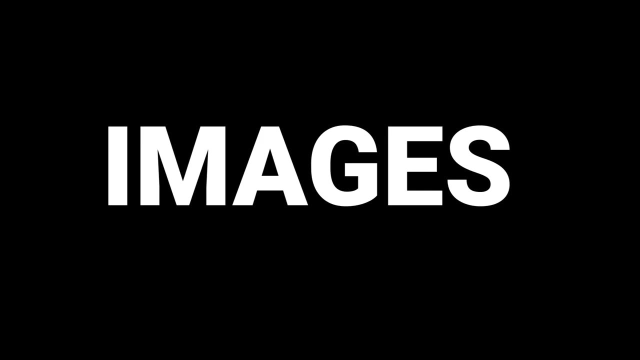 about a ul ol and then the nested list. so i'm going to select all of that, i'm going to delete all of them, and knife is so there and boom, everything is gone from our body, right here now. the next thing which we are going to be learning about is something called images. 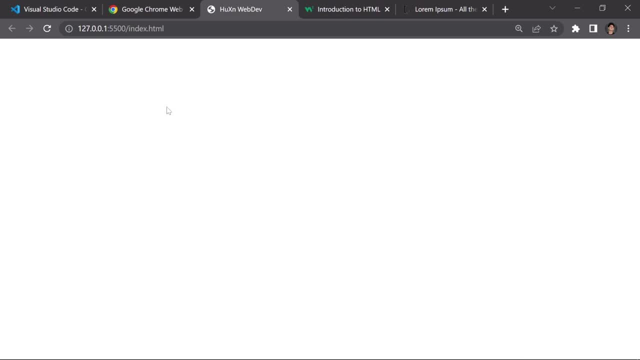 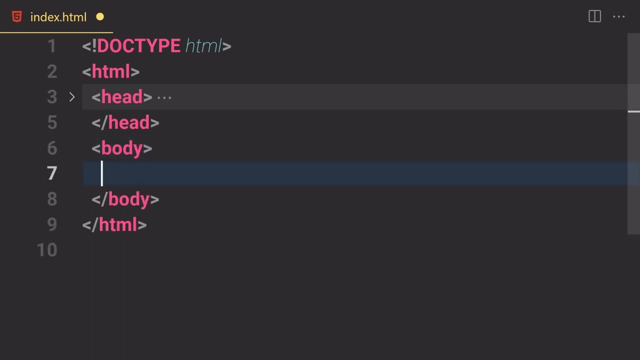 is that? how can we render our images into a browser? it can be either our own images or it can be some other image on the internet. so how can we render images into our browser? so for that we are going to be using img tag. so there are two ways to render your images. the first way we are 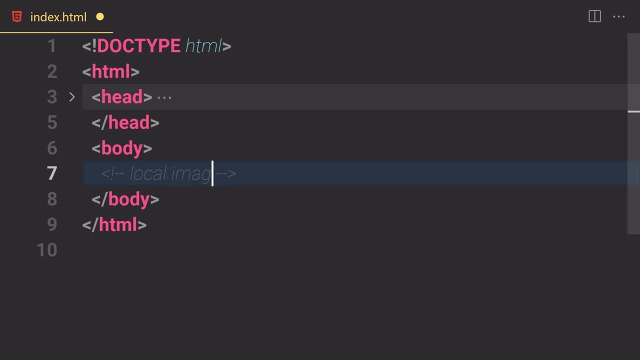 going to be learning about in this video is something called a local images, okay, so those images like those images which are currently available inside your machines. and then we are going to be learning about remote images, those images which are not inside your machine but somewhere on the internet and you have access to that like maybe you just copy a link from somewhere. 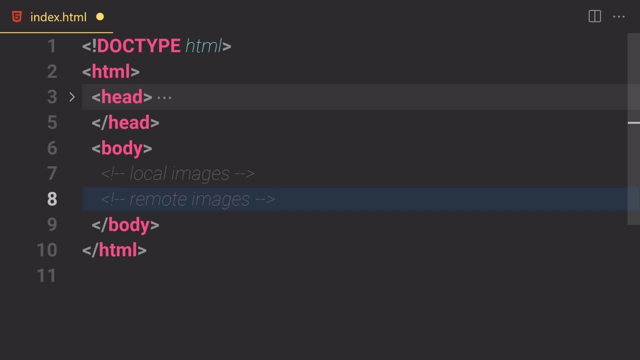 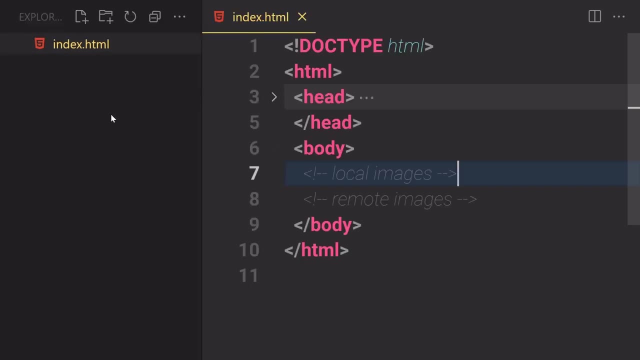 so we can also render that if you want to. so first of all, let's just learn about our local images. so for there, we would need to download an image into our machine and then we have to place that inside our directory and then we can work with that. so the best places, in my opinion, to find 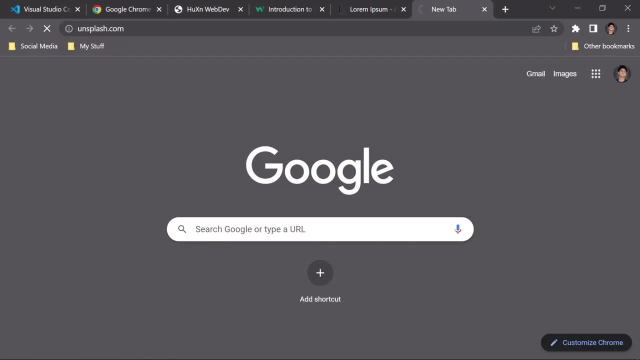 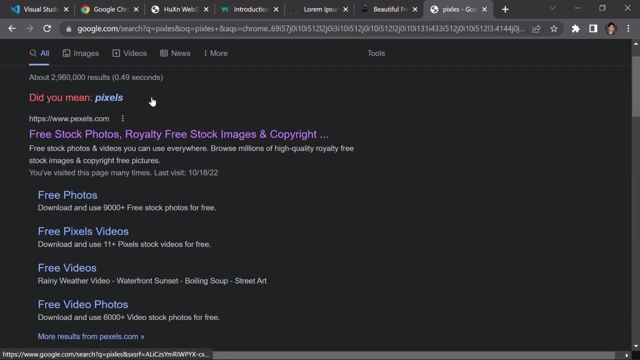 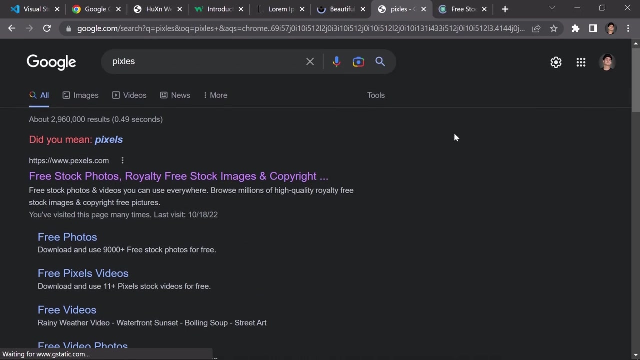 images are two places. the first one we have is unsplashcom and the setpixelscom- or just a pixel would be fine, so i'm going to just search for that and i kind of forgot it's your. and here you can see we have wwwpixelscom, so we can just click on that one and boom, it will open it right. 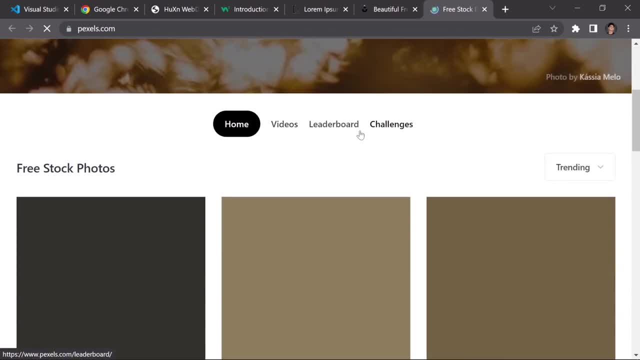 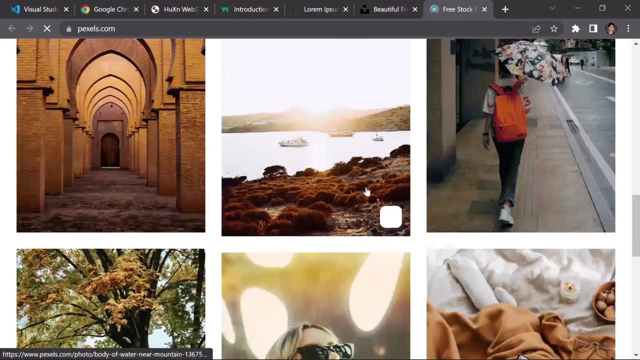 here and you can also find like videos and stuff like that. so we can just search for images if you want, or you can also choose it from here. uh, i don't know what's happening to my internet. it's taking a bit of time to render these images. anyway, so we can. 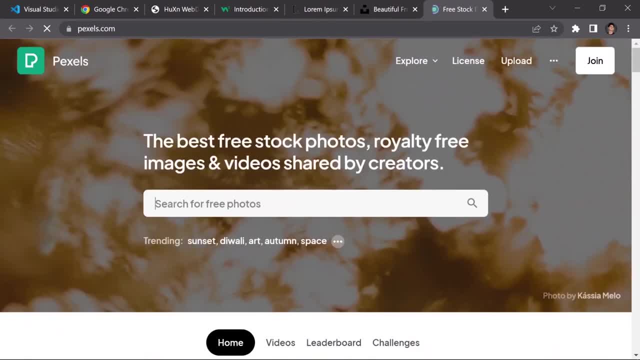 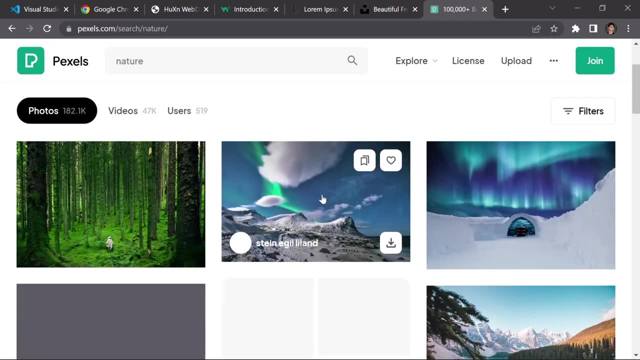 just choose images from here, or we can just type our own images. uh, for maybe, like a hacker or hacking or you know, i'm going to just search for nature, so i'm going to just hit enter right now so it no longer uses all of the nature images right here. okay, so you know what all of them are. holy crap. 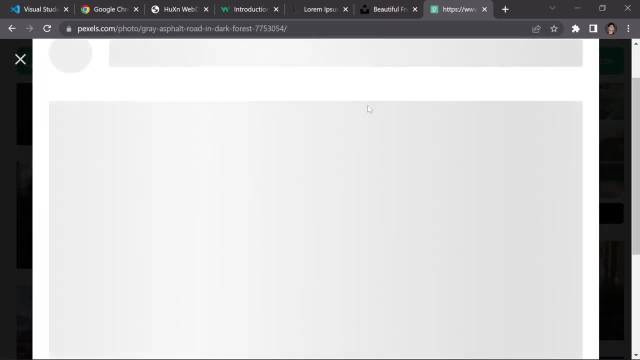 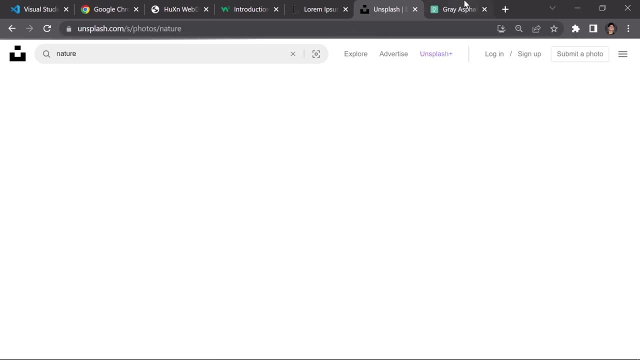 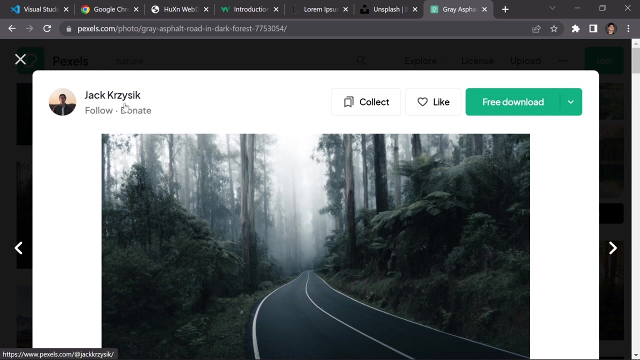 i'm going to click on this one because i really like a dark, and i'm going to also search for images in this tab as well, so i'm going to just search for a nature, nature. okay, so it no longer uses this image and shout out to this person: jack uh, craziness, sorry. 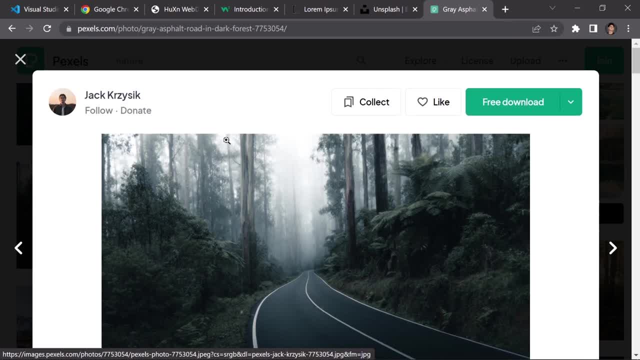 i can't pronounce your name, buddy, and in this course i'm not going to be pronouncing people's name, because in some cases i do mispronounce people's name and then i feel weird about that. so i'm not going to be pronouncing anyone's name in this course anyways. so if you want to download, 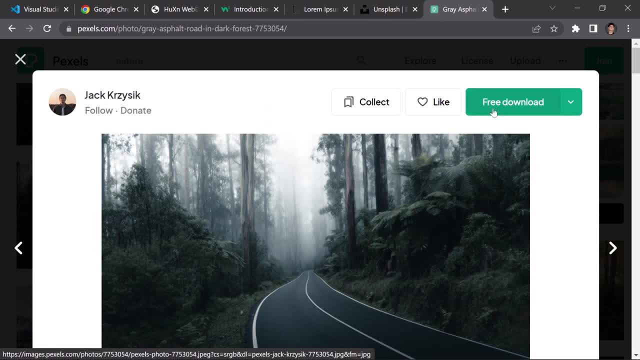 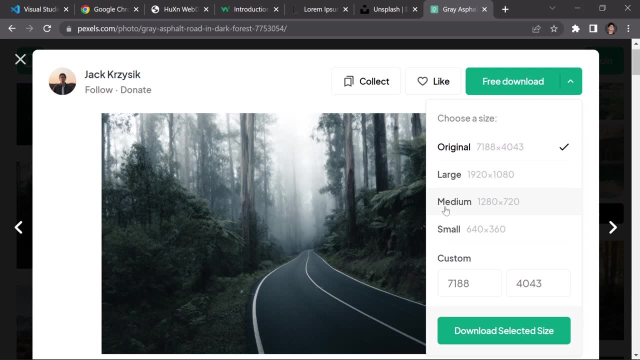 this image. you can just click on download and you can also click on this icon, and you can either download the original size or a large size, the medium one or the small one, or you can also write your own customized size if you want to, but in my case i'm going to just uh, click on this one. 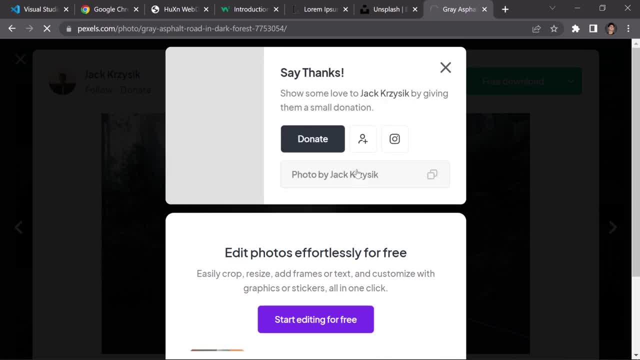 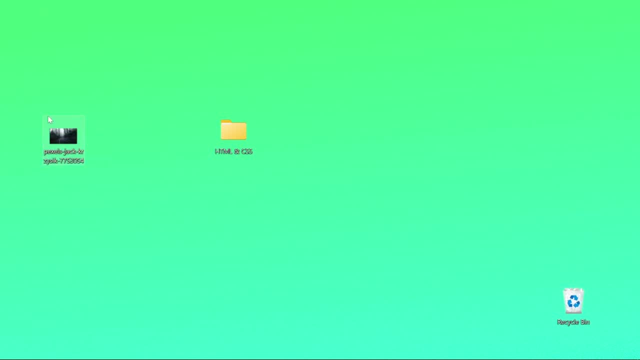 or you know what? we just have to click on this download button. so now just download this image into our machine. all right, so now that we download this image right here, so what do i have to do? i have, and by default it went to our downloads folder, so i'm going to just grab that from here. 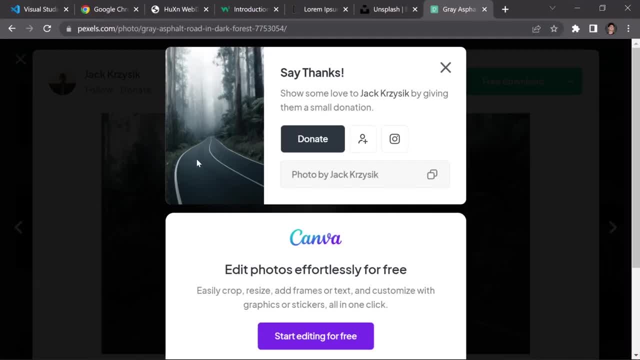 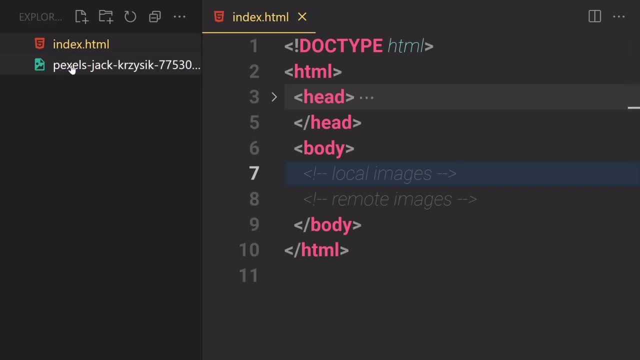 and i'm going to put it inside this html and css folder. and now, if you open our visual story coder, and now if i hit ctrl b right here, so what do we have? we have this image right here. so if i just click on that and it will now open this image in our visual story coder. 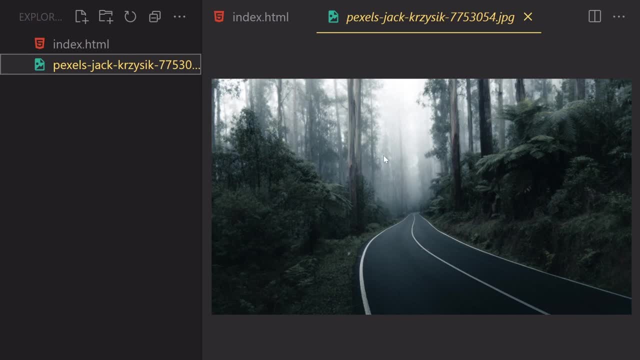 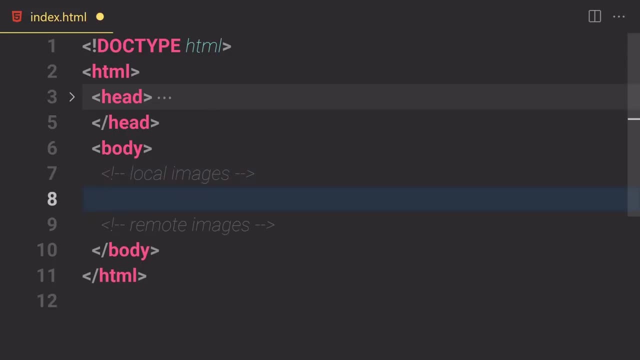 and this is how it looks like right now. now, if you want to render images into our own website, so for that we can use just img. so if you just write like img and if you hit tab, so it will now gives us a few things. first of all, it will give us this img tag right here, and then we have two attributes. the first: 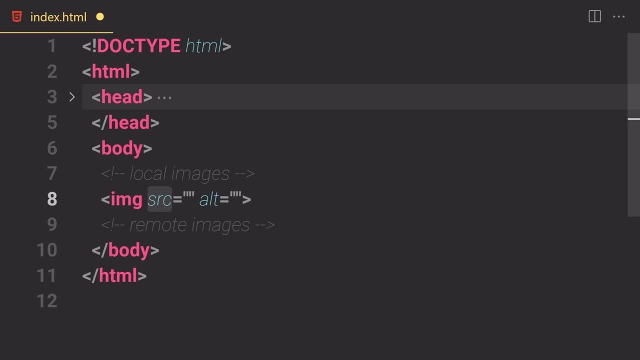 attribute, we have a src and which stand for source, like the location of the image, and then we have a alt and this art stand for the alternative text, like: if this text, like: if this image is available, so show this image. so, if this image is not available, then show this alternative text and you. 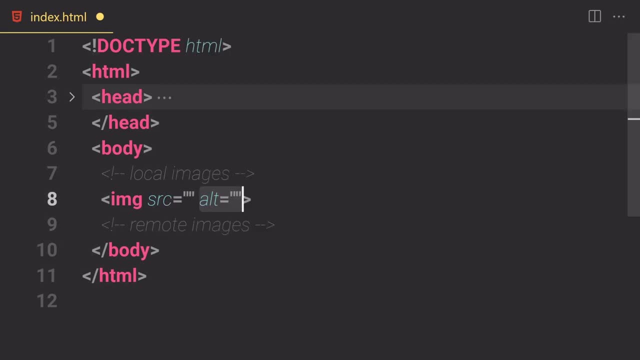 can also remove this alternative text if you want to like, if you don't want to like, if you don't want to provide alternative text for your image, so you can also go with that. so now, if you want to render your images, first of all you have to provide the url or the link or the location of 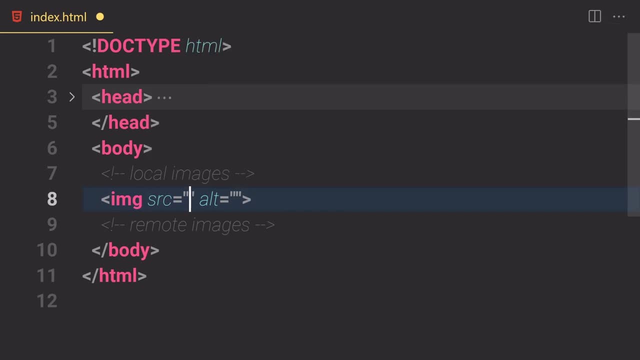 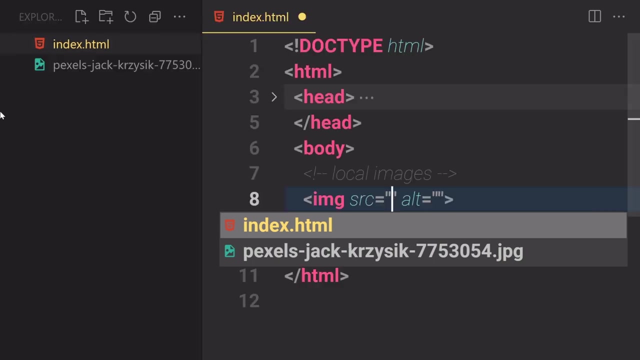 your image inside this src and then in these quotes right here. so now that we know that our image is currently available inside this directory, like inside this folder. so for that, what do we have to do? first of all, we just have to hold ctrl and then have to hit space. so here you can see. it all now shows us all of the files and folder which are: 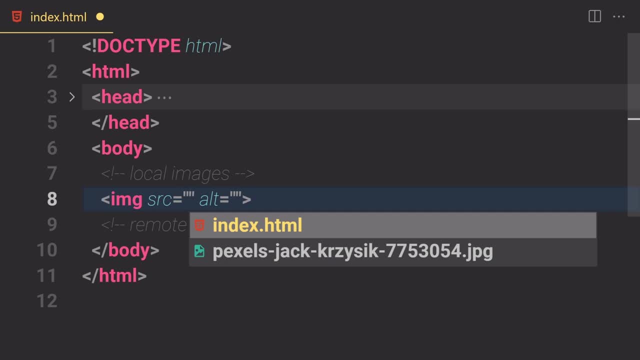 currently available inside this directory right here. so by default or not by default, but currently we just have this indexhtml file and then we have these pixels and then this image. so i'm going to just select this one, and now, here you can see, this is the actual url of that image. okay, so for now we 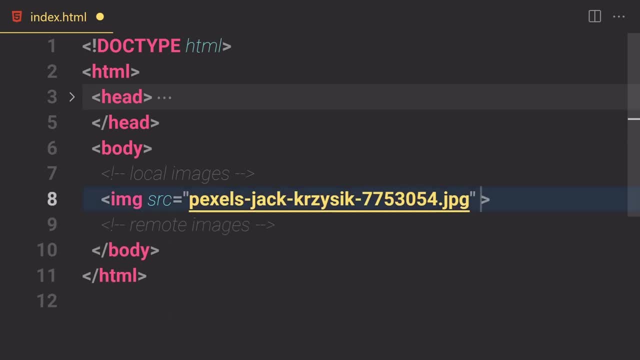 are going to be just removing this alternative text from it. so i'm going to just remove that. and now here we just have to close that by just providing a forward, not a forward slash, but just a slash right here. so now if we save our file and boom, here you can see, we have that image. 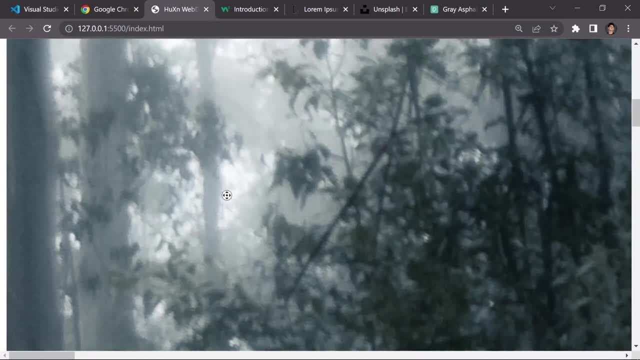 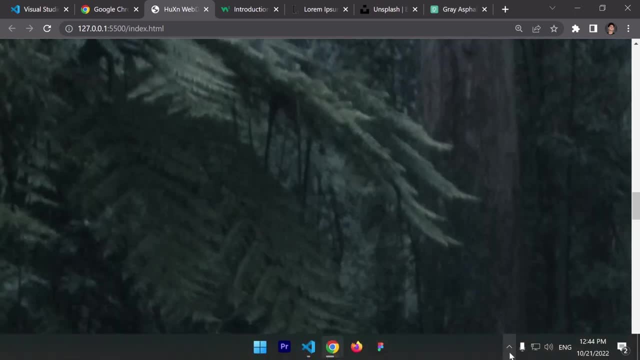 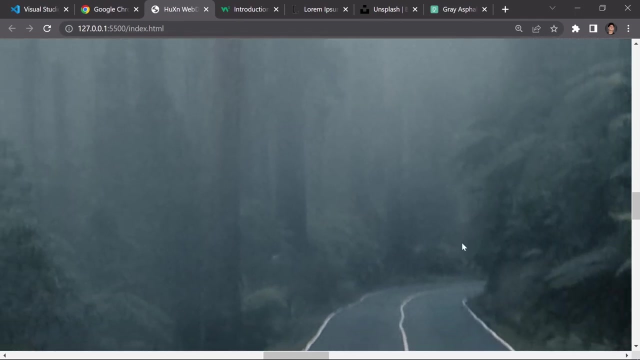 but it is supremely massive right here, like we cannot see even the road which used to be inside this image. let's just say, oh my goodness, it's too much, okay, it's too big right here, arts, now we are inside in a road, now we can see that. now, if you want to give like maybe your own width and height, 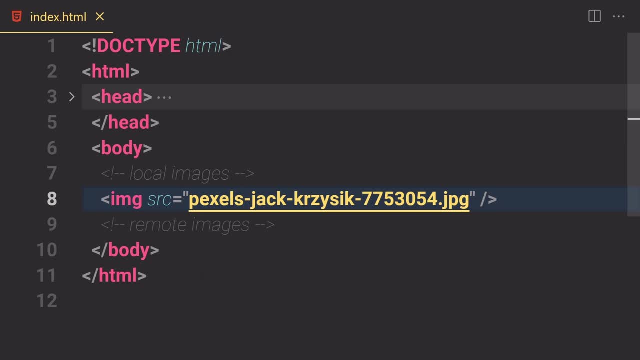 so for that we can provide our own width and height right here. so we can provide our own width and height here, but this is not the best way to provide a width and height to your images, and later in this course we are going to be also learning about how to provide width and height by using css and 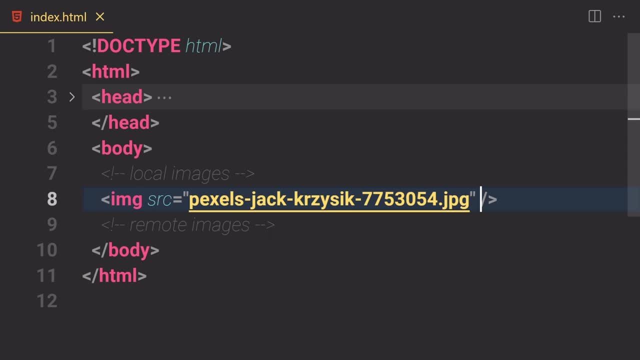 css is a new technology which we are going to be also learning in this course, but for now we will just go with the ugly and crazy way. so we just have to first of all write like a width, and if you hit tab, certain log uses this equal to sign, and then this double quotation if you want to write. 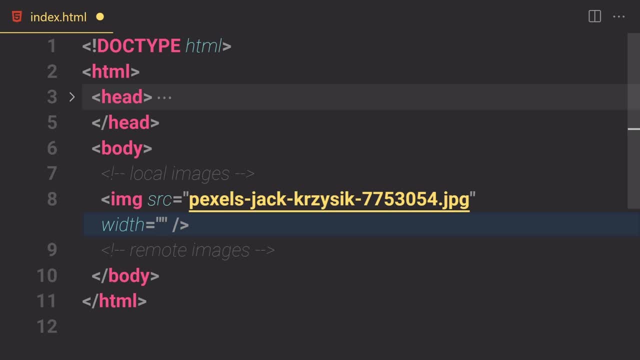 it manually. you can also write it manually, so now let's just specify how much the width should look like. so we just have to apply like 200 pixel, and you don't have to worry about these pixels for now, but you just have to type it right here. i want you to just type it, and now here we just have to. 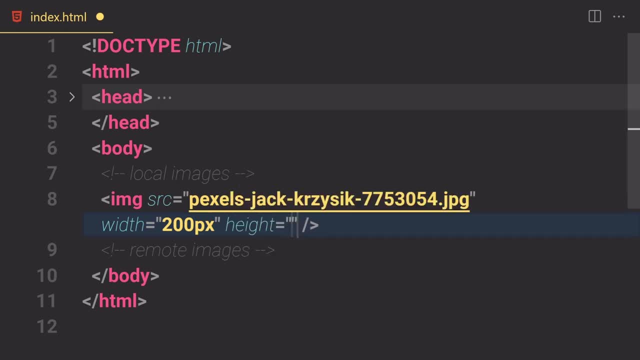 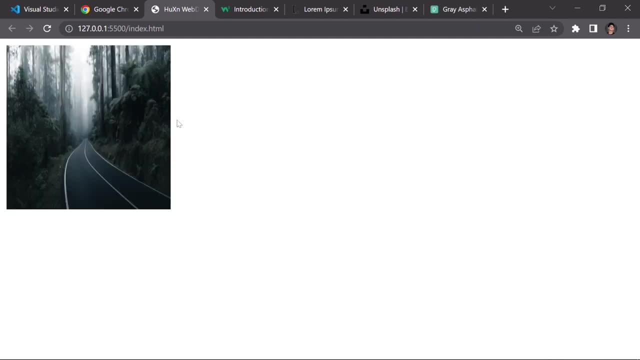 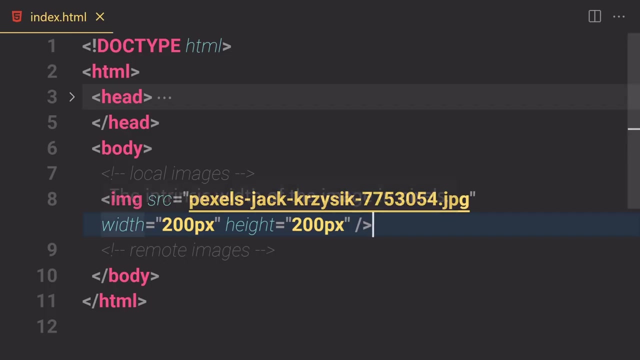 place our height right here. and if you hit tab and we also have to give him some sort of a height, maybe like 200 pixel in this case. and now if you sell file and boom, okay, it will take a little bit of time, and now boom, here you can see, we have our image 200 by 200. you can increase or decrease the. 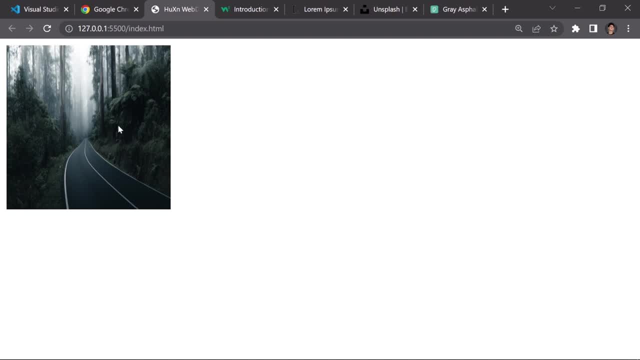 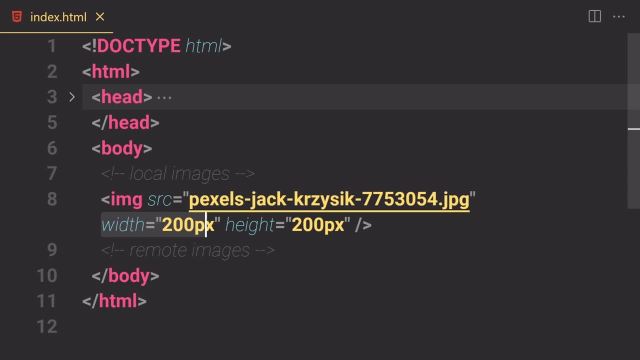 sizes if you want to. but now, congratulations, we successfully rendered image into our browser right here. okay, uh, okay, so this is kind of the bad way to write your width and height. first of all, let me just say that, and we can also write alternative text, but we will write alternative text for the scenarios like these one, let's suppose. 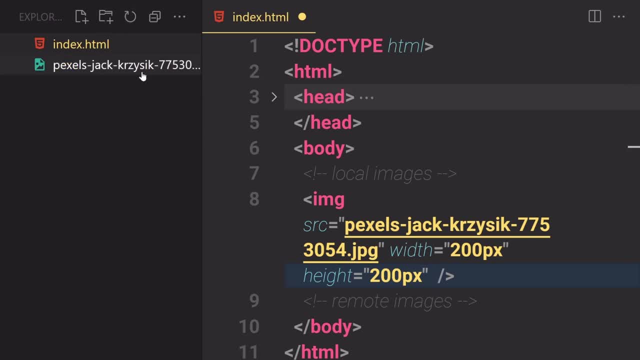 if we create a new folder. and, by the way, if you want to create a new folder in a visual story coder, you just have to click on this uh folder icon and here you can see it will not use like our icon right here, so we have to specify some sort of a name right here. so in my case I'm going to 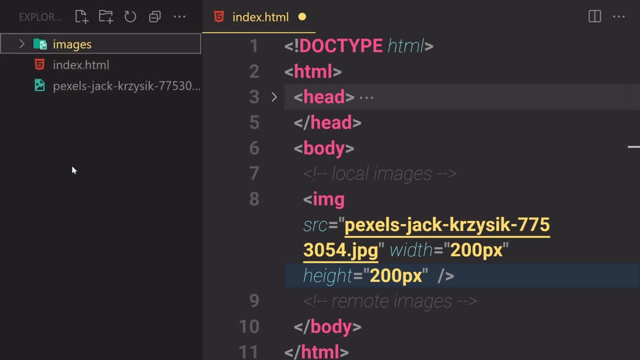 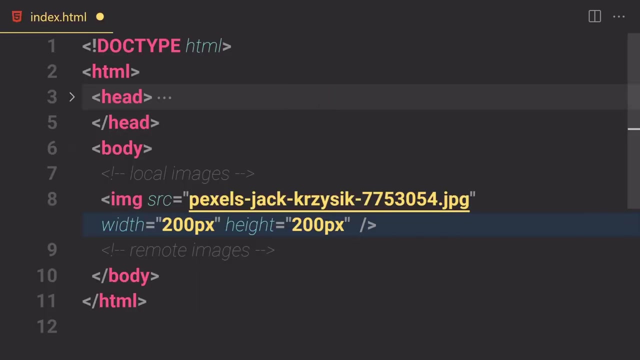 just give my name of like images. and now, if I hit enter, and now we just have to grab this image from here and now let's just push it inside this images folder. okay, so now our image is currently located inside this image right here. so what is break inside our code? okay, so now, if you just save our 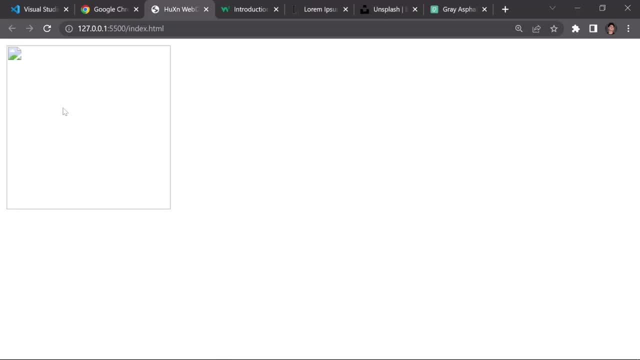 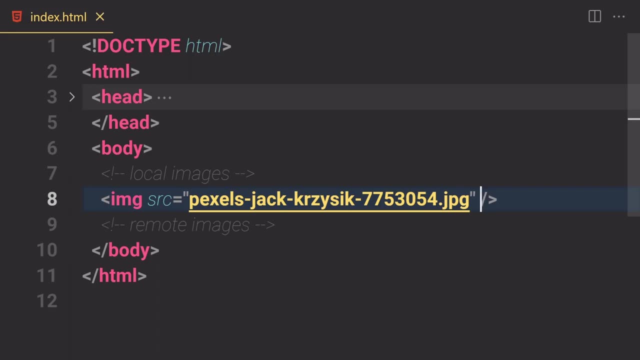 file and here you can see our code breaks right here and we are getting like a width and height provided right here like manually. so if you just cut there and if you save our file, so here you can see, it along uses kind of a broken image right here, which means like nothing, like no image. it. 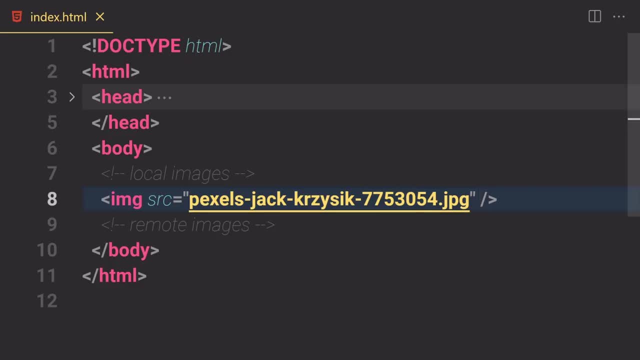 used to be an image in here, but we don't have that image available, no more. okay, so for that we can write or alt, as we saw just a beginning of this section, like alternative text, so we can just provide anything we want. but we're not going to be providing anything we want, so we will just 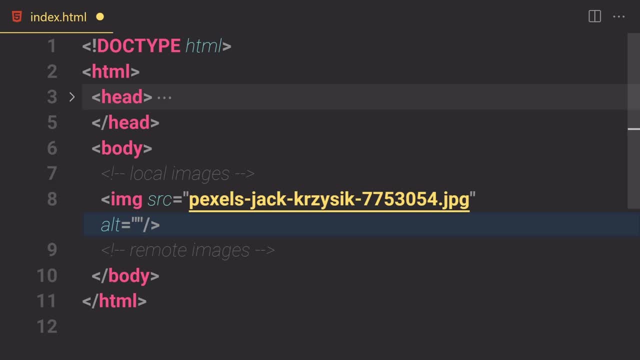 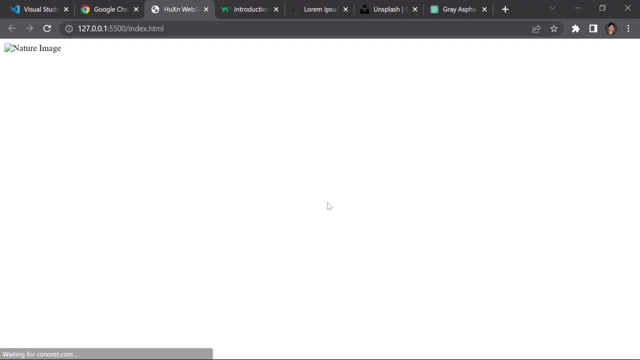 provide some sort of a message based on that uh kind of image. so in this case I'm going to just write like nature image or used to be a nature image. so we would just save our file and boom, here you can see, we are now getting this. 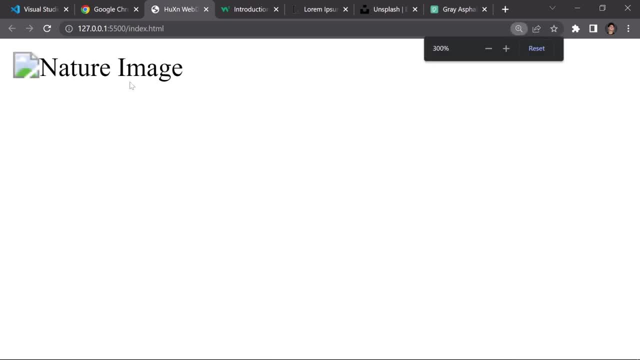 nature image kind of text right here and it will tell the users like your internet connection is wrong or something went wrong in this website. that's why we are not getting that image. but here you will see the nature image, okay, so we are just telling that kind of like a message to. 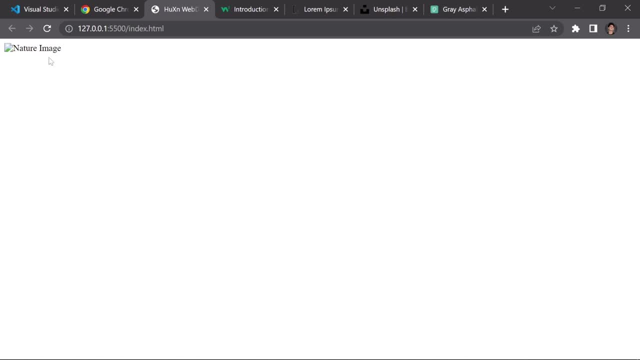 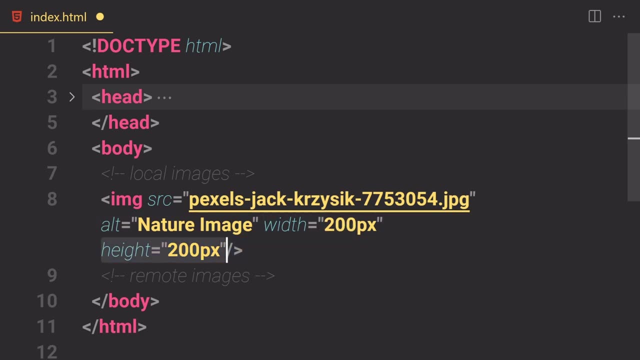 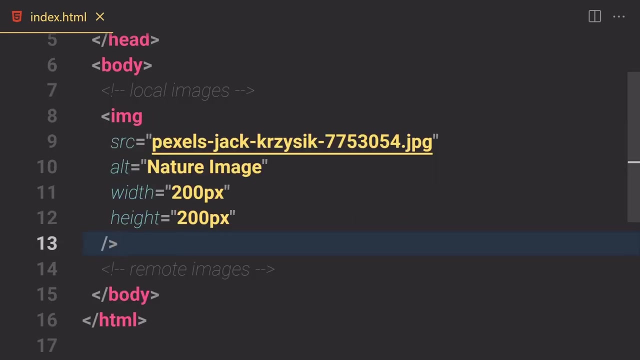 our users, like here, used to be a nature image, but we don't have that image available for some sort of reasons. so we can also provide our width and height bank, like 200 pixels by 200 pixel height, and if you save that and just, it will not do anything for now. okay, now we do provide our width and height. 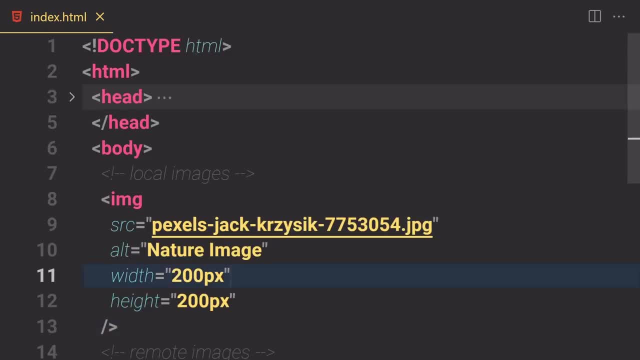 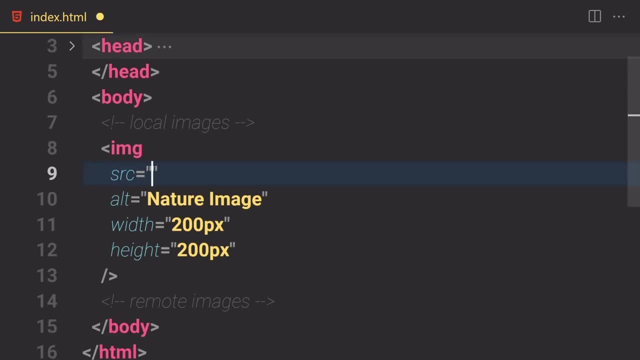 right here, but we don't have that image working. now, what do we have to do to bring our image back? so, first of all, we just have to remove all of these stuff from here and now. what do we have to do? I already show you the shortcut, but if you forgot in some case, so you just have to hold. 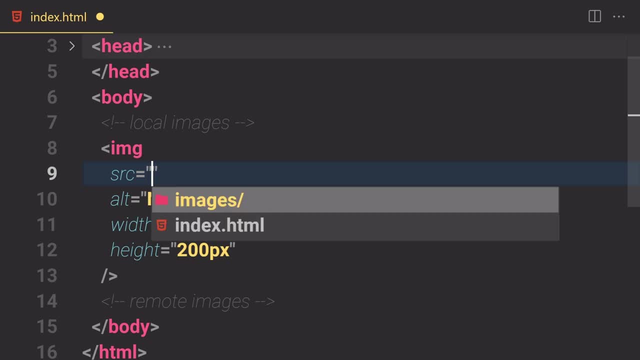 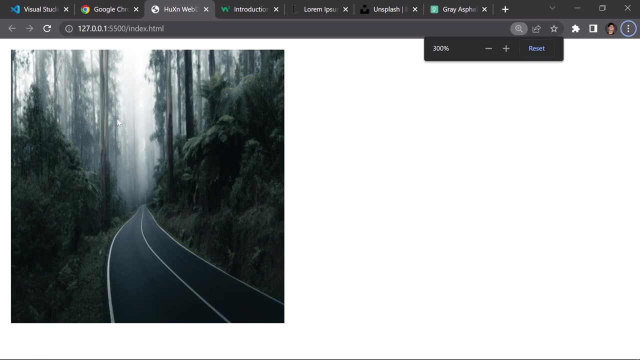 control and if you hit space, everything which are currently available inside this directory, so we will just select the images folder. then inside this images folder we have this image right here. so if you click on that and if you save our file and boom, it will now brings us our image back right here. okay, so 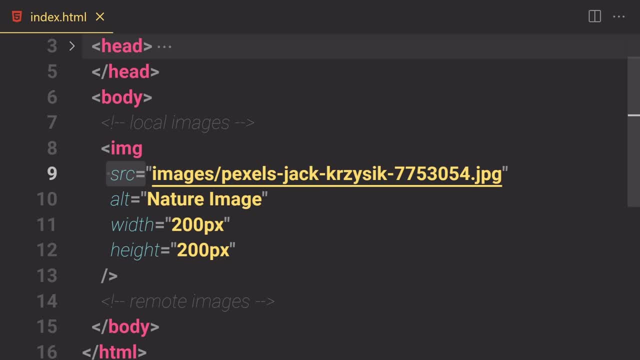 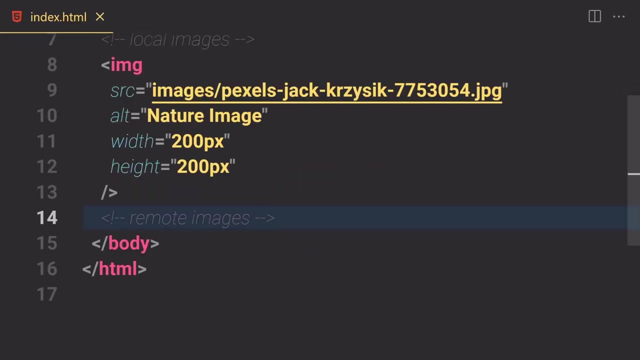 and this is how we can work with the paths like this is a SRC, like a source, the alternative text, the width and height. you also learn about width and height. so this is it, about a local images, like those images which are currently available in your machines, right here. so now let me just show you the remote way of writing your 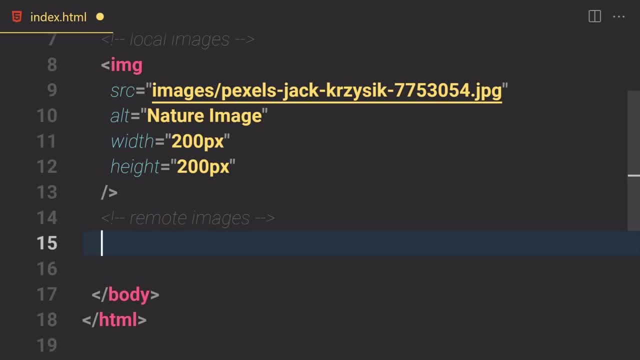 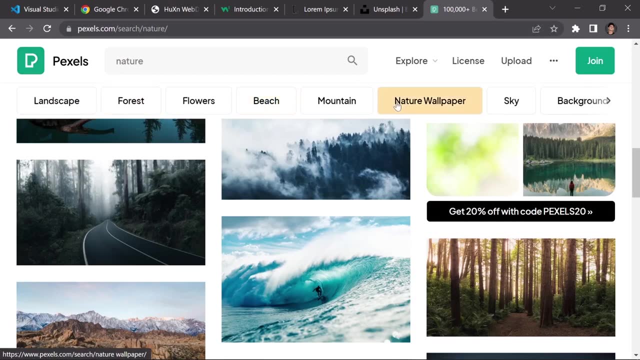 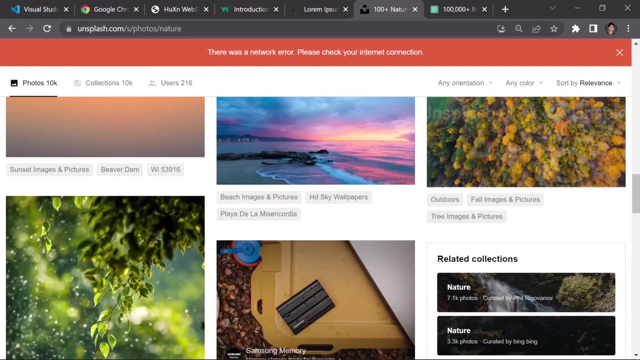 images, so how it will be looking like. first of all, we will need some image to grab first of all. so for that we can just either go to this pixels website right here, or we can also go to this unsplash one. so here are awesome images I'm gonna click. oh, okay, I'm gonna close that for now anyways. so I 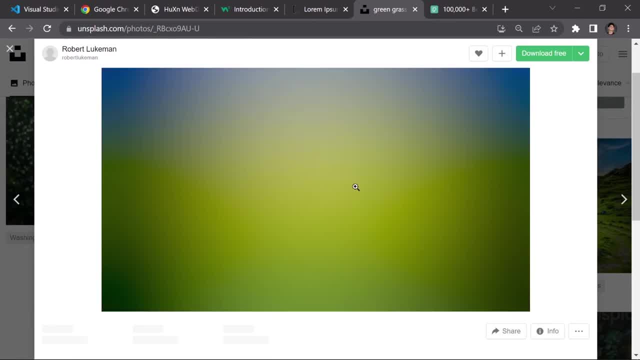 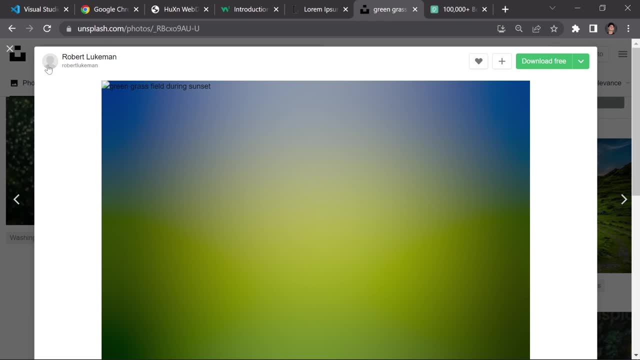 don't know which one should I pick. I'm gonna click on that one and then: okay, so it's not really here. you can also see that's because my internet problem- and here you can see this image- is broke and we can all see this guy image as well. so I don't know. 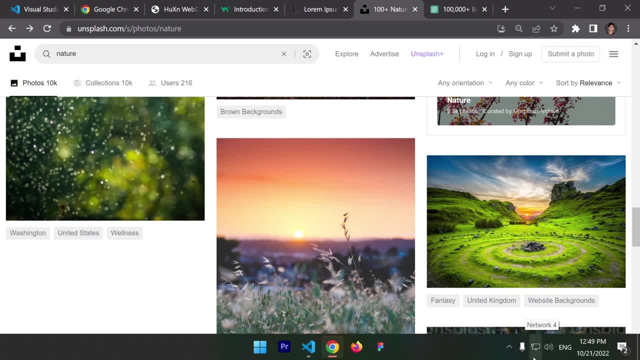 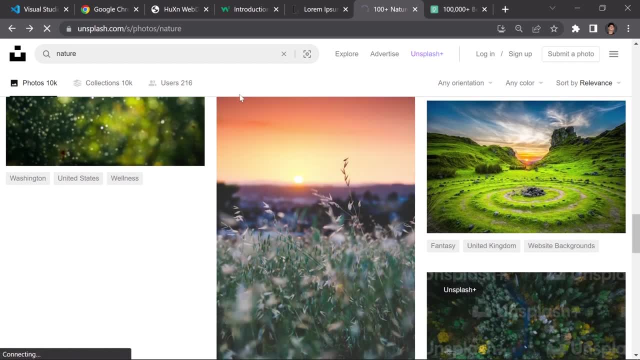 what's up with my internet connection. let me just see that, okay, network, it's connected, but I don't know why. just refresh my browser one more time so that we can see the speed of our internet. okay, so we are back. my internet was so, so low. I don't know what happened, but you know, what I'm gonna do is I'm 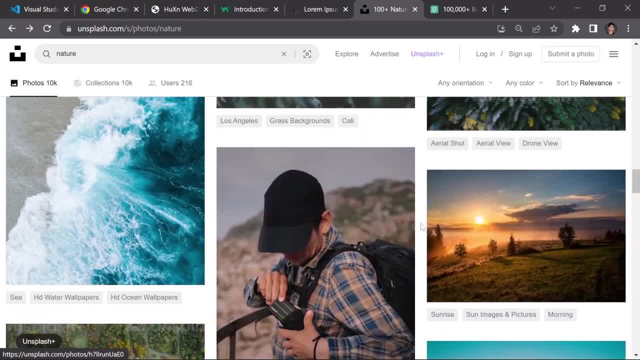 gonna turn on because it's because let's see then again, if I turn off the backs on this page, we want to see if we can see them. ok, so what we did was that the speed of our white facebook messages was an instant up, but you know what kind of thing I don't actually remember to incorporate this movie using it. well, 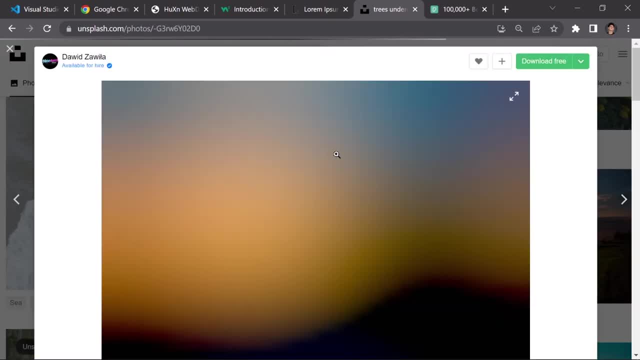 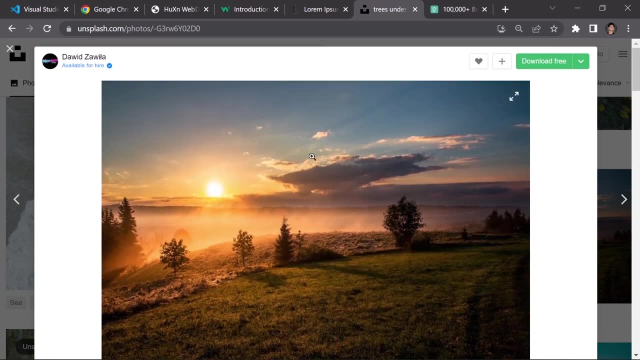 you know, i'm going to just click on this image for now, so it's taking a bit of time- and shout out to this person and he's available for hiring if you want to hire him out. so now let's suppose we just like this image, so we just have to right click on it and then not a copy image, but a copy. 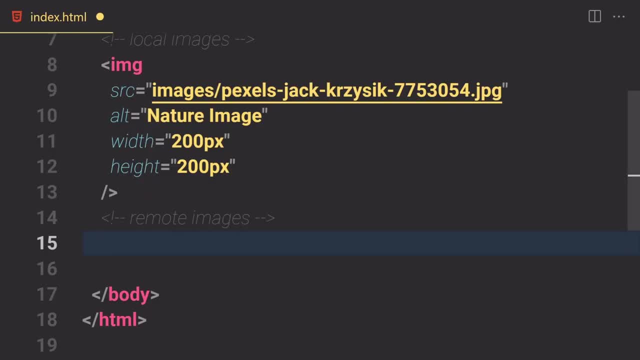 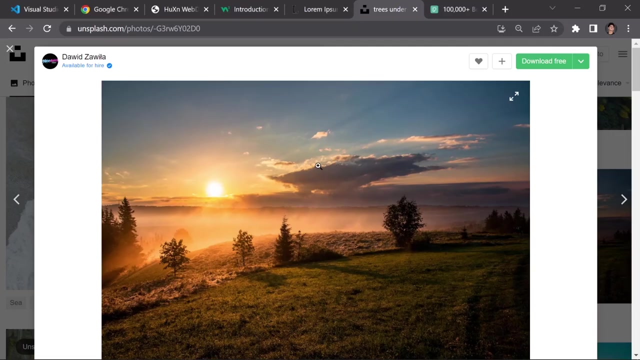 image address. so we just have to click on that and then go towards css or not css but or html file. but we just have to write img and if you hit tab and now inside the source we don't have to write like hold, control and space and stuff like that. here we just have to paste that image address. 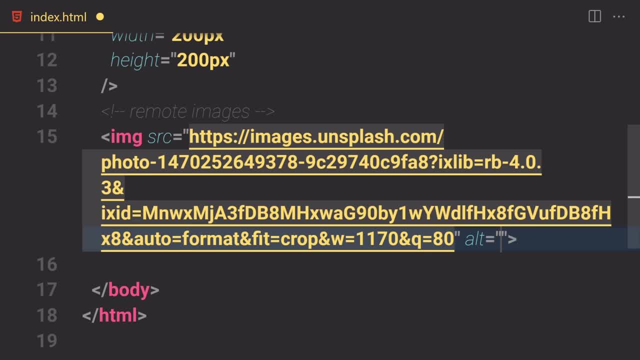 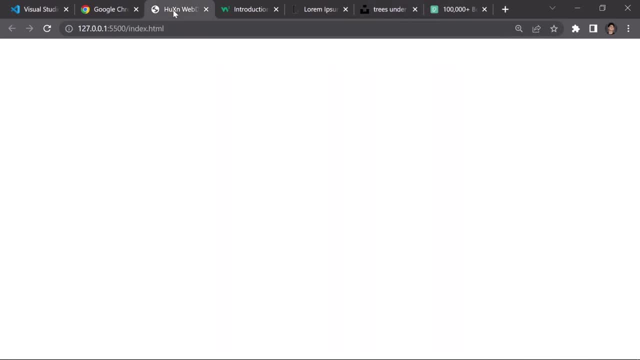 which we just copied it from here. and now, here you can see, we have that image address and we are not going to be providing anything for the alternative text. so now, if you save a file, and now here you can see, we have this massive image. if you want to make that smaller or bigger, 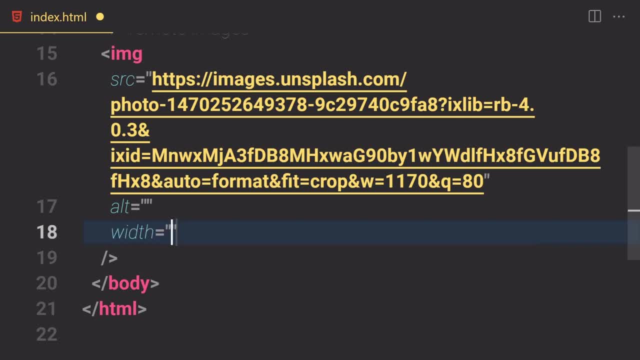 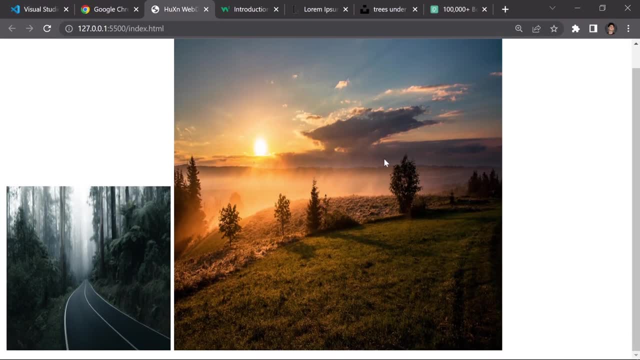 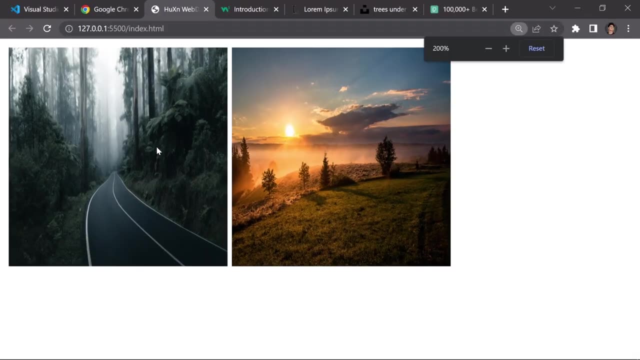 so for that we can write or attributes like width of maybe 400 pixels and height, also 400 pixels. i'm going to send my file and here you can see. this is how it looks like, so you know what i'm going to provide- 200 by 200, so both of them look the same. so here you can see both of them are. 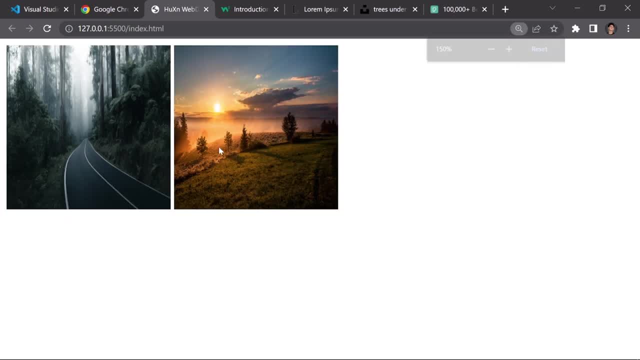 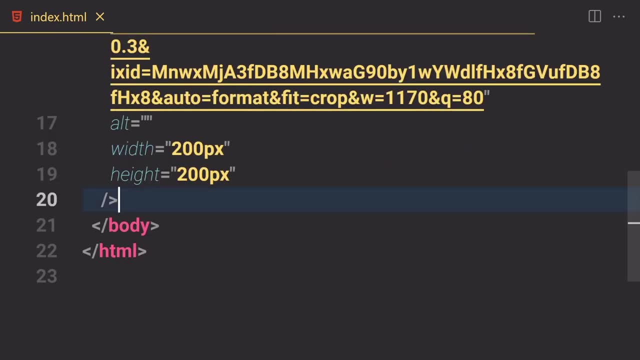 looking the same, and this is how we can render images using our html. so that was it about, for remote images and also for local images. but i just kind of want to mention one more thing. i'm going to remove both of these images from here and now. let's just talk about something. 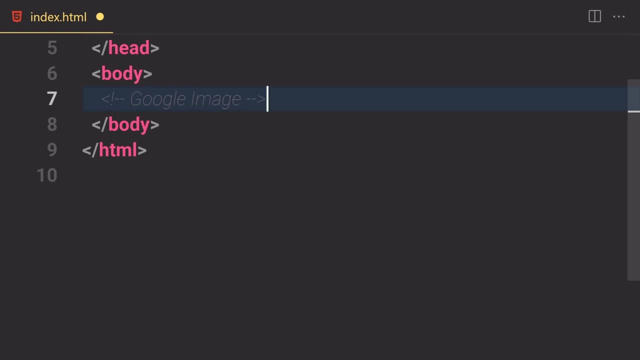 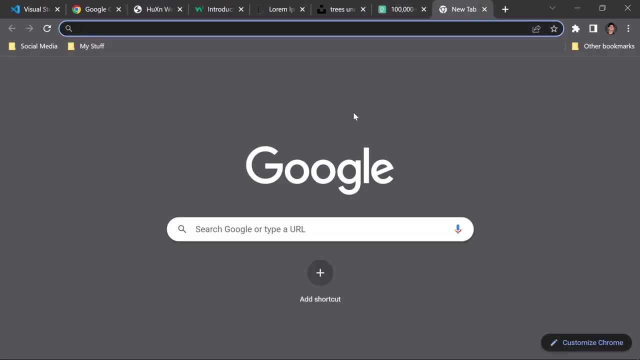 google images. you might be also thinking like: uh, hussein, we already have a google images, so why do we have to search for unsplash or, uh, the pixel ones? so now let's just, uh, go to the google images. uh, maybe i'm gonna just write nature in here and then we have to just 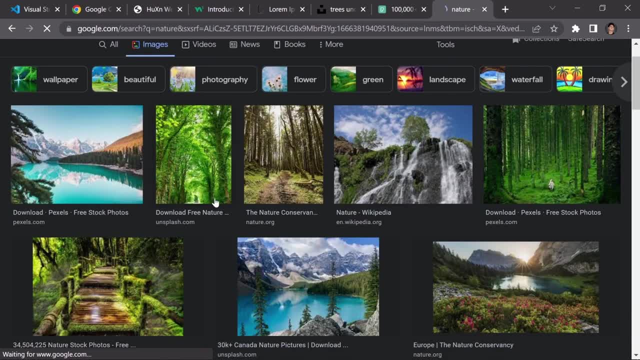 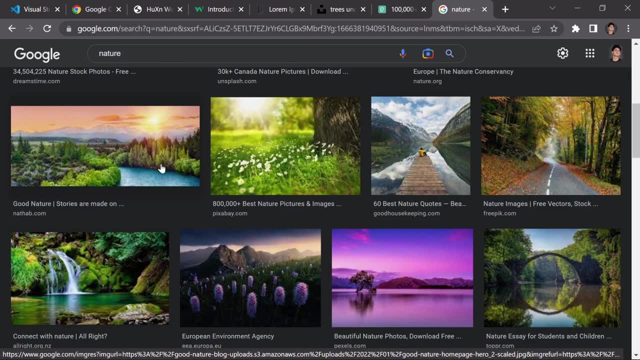 go to the images right here and now. here, let's suppose, if i want to select- maybe- i don't know- i'm going to select this image. uh, yeah, i'm going to just click on this image, or you know, i'm not going to be clicking on that, i'm going to right click on it and then here you can see, we have this. 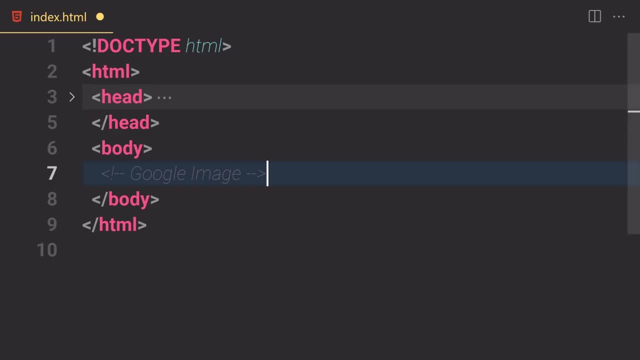 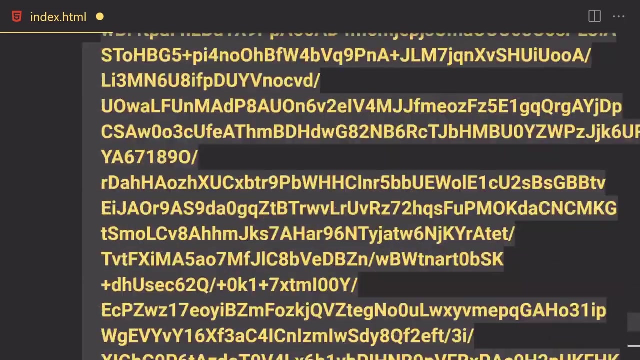 copy image address. so i'm going to click on that and now let's just render that. so if you want to render that image, so for that we are going to be just writing like img. and now just i want you to just notice there. so if you hit ctrl v right here and boom, okay, so look at this crazy url right here. 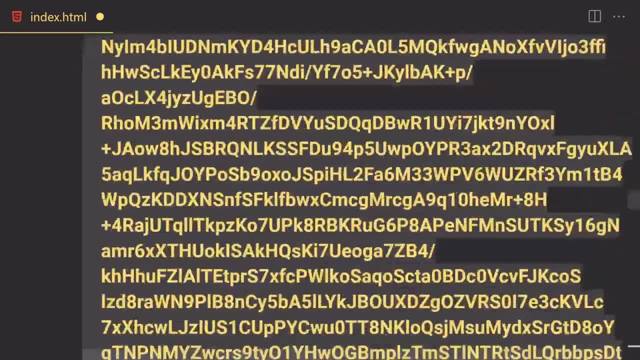 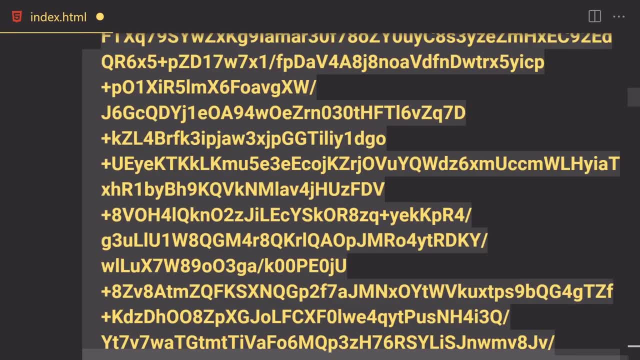 so this is why you are not going to be using a google images. look at this url right here. so it's supremely massive. now you might be asking, like who's that you have zoomed in a lot, so you just have to zoom it back. no, we don't have to zoom back. this is a really long url. so if i just 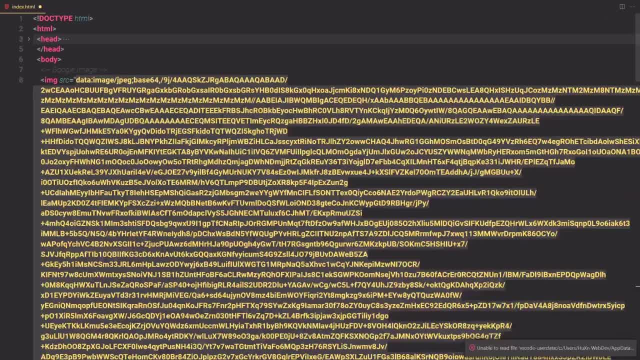 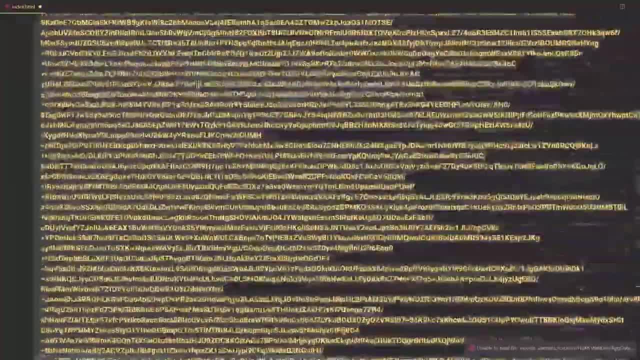 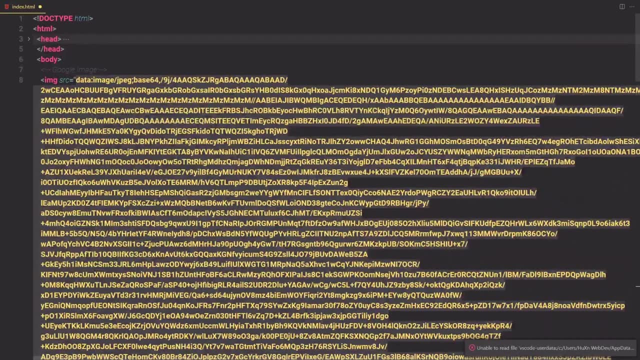 maybe zoom out like zoom back, back, back, back back. so here you can see. this is how the google images url look like. oh my god, it's supremely ugly and nobody will wants to work with that. it's kind of like a svg, or maybe it's thousand time longer than svg and you don't have to worry about svgs. 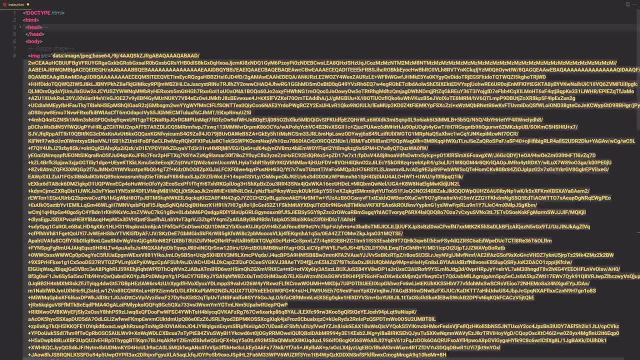 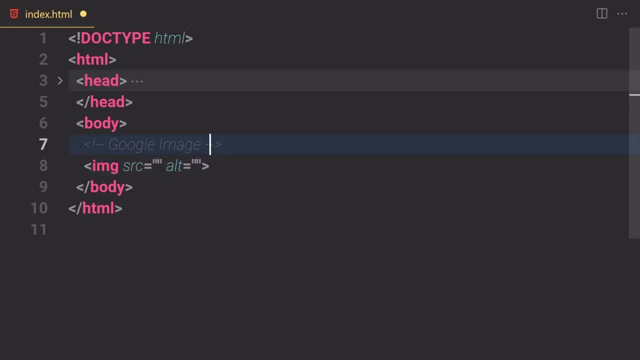 which we are going to be also exploring in this course. but what do we have to do? we have to just undo this step. and now, uh, my recommendation would be to never, never, use a google images. so there are two ways. the first way that we already saw that the url will be supremely. 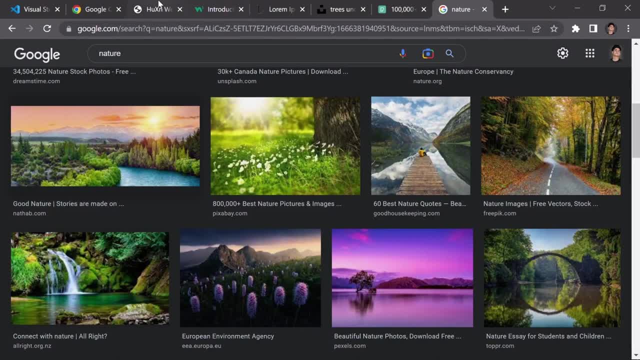 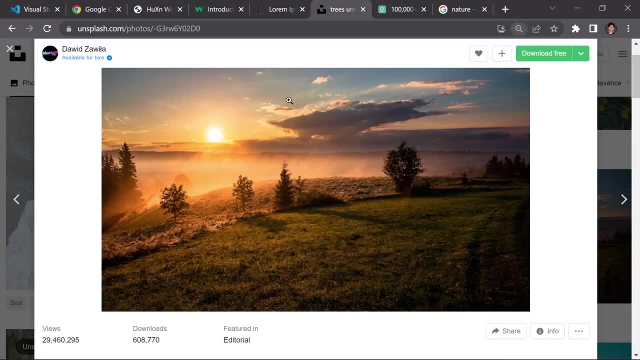 long. so if you just put this url in here and if you save our file, so it will gives us that image right here. but look at the quality of this image. i mean, like, look at, it's supremely awful. let's suppose if you want to like, uh, render this image, so we just have to copy that like a copy image. 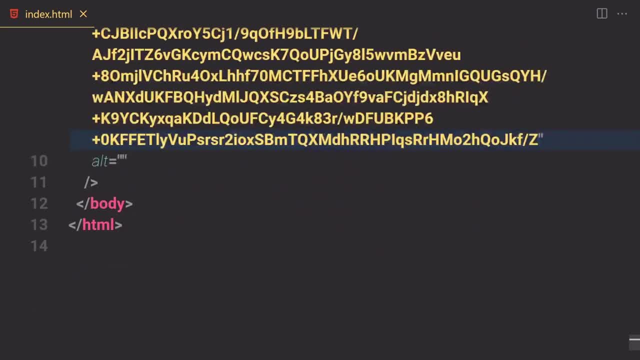 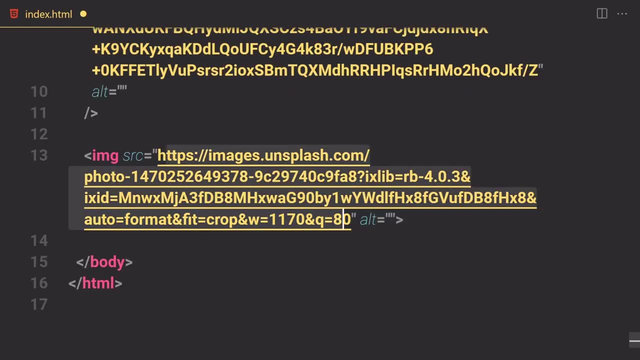 uh address. and now let me just render this image as well right here. so let me just write image and here i want to paste this link, so here you can see the image. so i'm going to paste this link. so here you can see like we have kind of a long url right here, but it's not that much like compared to this. 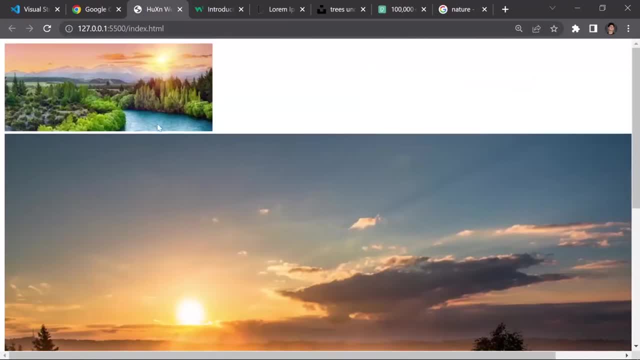 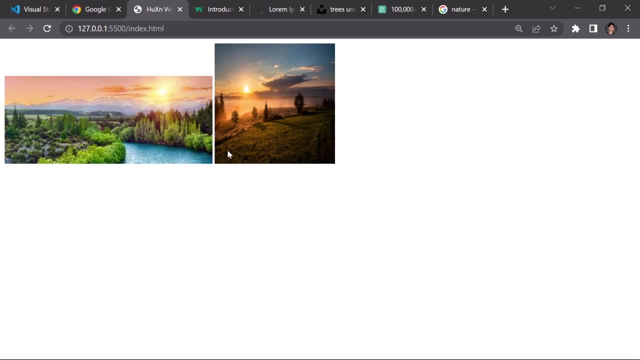 one. so if you save that and here you can see it along this high quality image right here. so if you just write like maybe, uh, width of 200 pixel and height will be also 200 pixel, if you save that and here you can see, i want you to just notice the quality, like like: this one is supremely blurry. 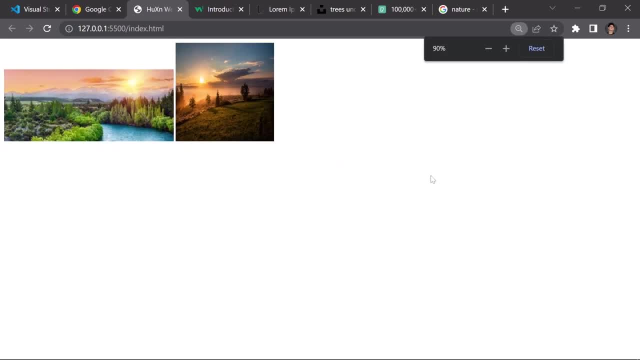 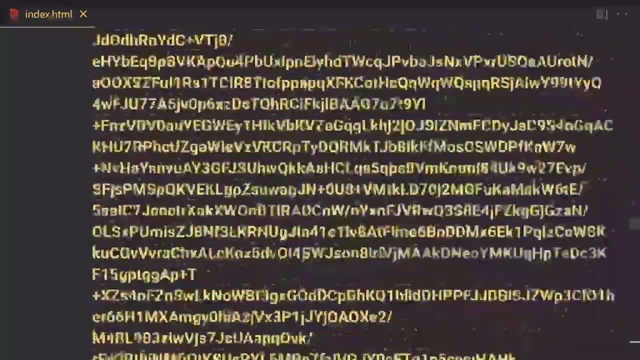 and this one is sharp and awesome. okay, so this is how you are not going to be using any google images and in some cases, the weird thing is that in some cases, they will just remove that image from google because you don't own that image. so never, ever use a google images. 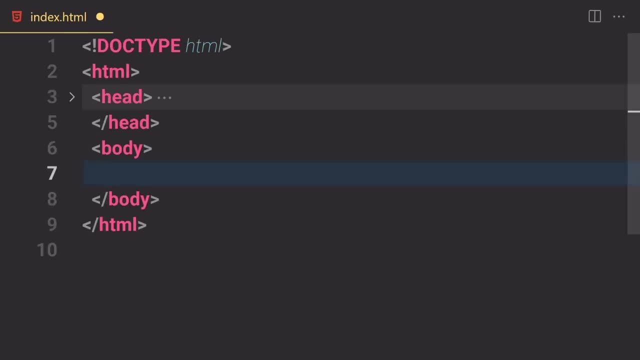 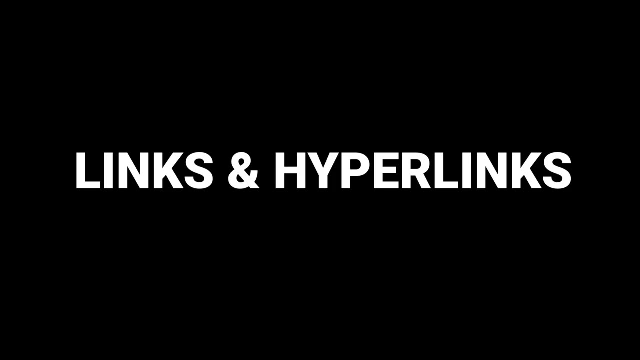 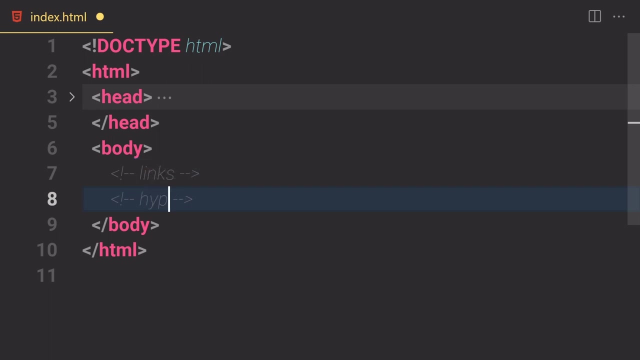 so i'm going to just remove everything from a body and i'm going to zoom in a bit, save our file and everything is clear. so that was it about images in html. now the next topic which you are going to be learning about: something called links and hyper links. okay, so in this video we are going 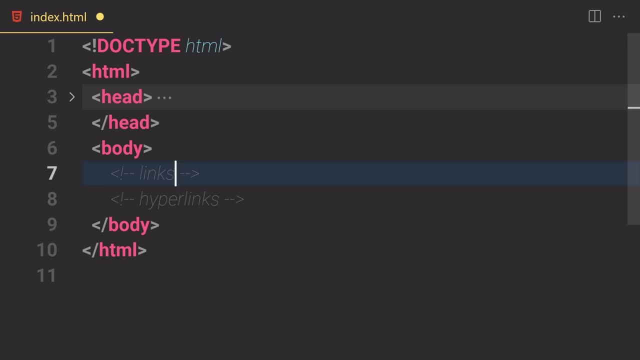 or not in this video, but in this specific section we are going to be learning about links and hyperlinks. what are links and hyperlinks? so a link, as the name suggests. there it will just link or web page to some other web page, like. maybe for some cases if i just write like uh, 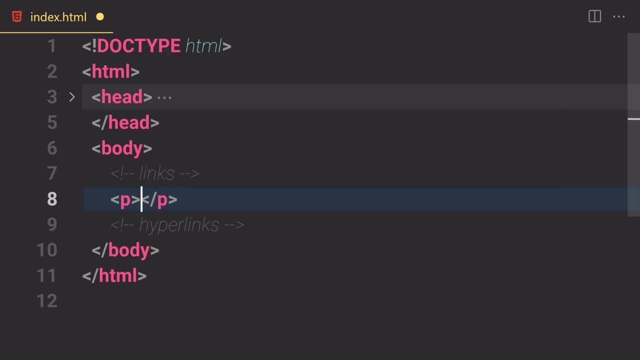 so for some cases, if i just write like paragraph and then let me just write like: uh, check out this awesome um site maybe, or you know what, check out this awesome game or whatever, and here you don't have to worry about this coding which i'm writing, but here we can also just place, and then we just 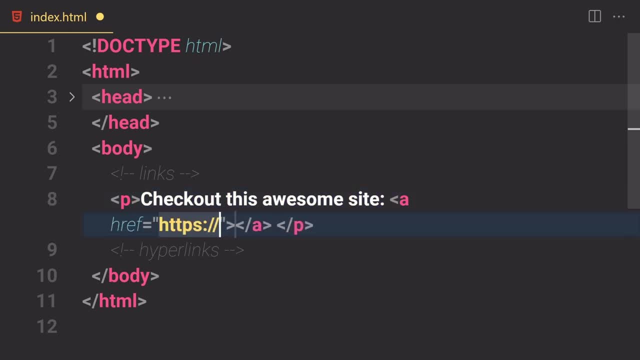 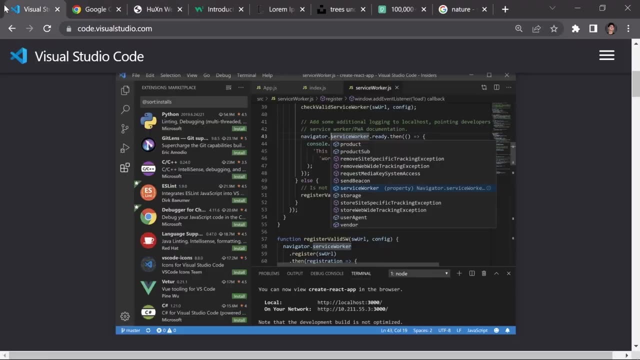 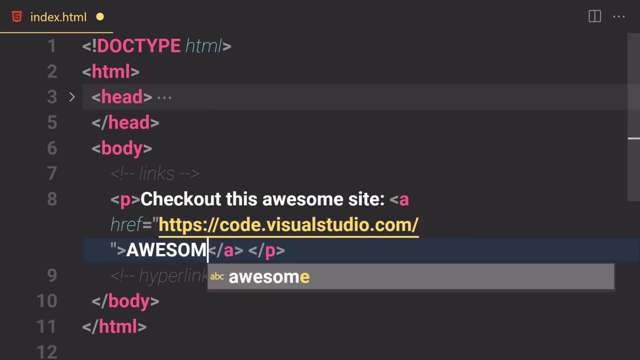 have to write like www or not https, then double colon, www dot, maybe some random site. you know, i'm going to copy this url or maybe this, this url from here and i'm going to paste this url right here and we just have to write like: awesome game, okay, so we can just record users. so if you just 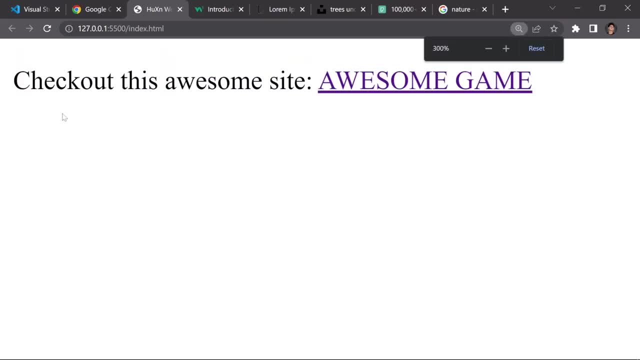 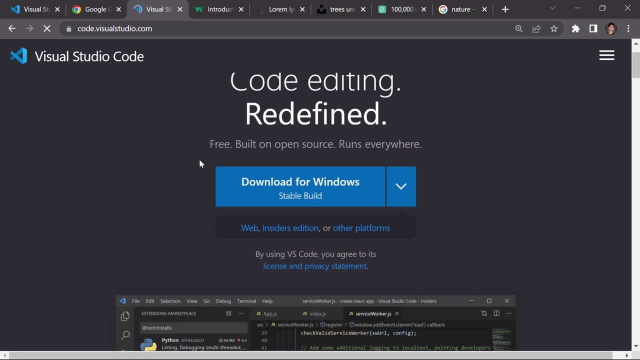 save our file and if you just click on that here you can see we have like check this awesome site. and if you just click on that and now brings us to a visual story coder, so this is a link. okay, and never use this kind of language in. 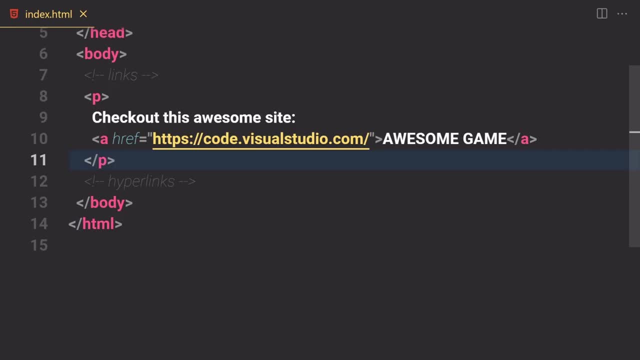 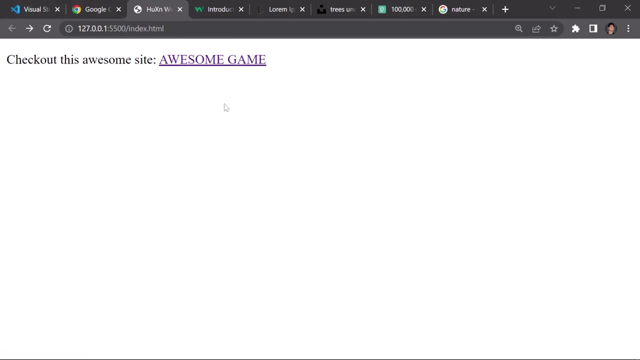 your sites. so this is a link. you don't have to worry about the syntax, but it will allows us to link from one page to another page in some sort of other server on the internet. okay, so it will just allows us to link to other website on the internet. so what is a hyperlink? a hyperlink will 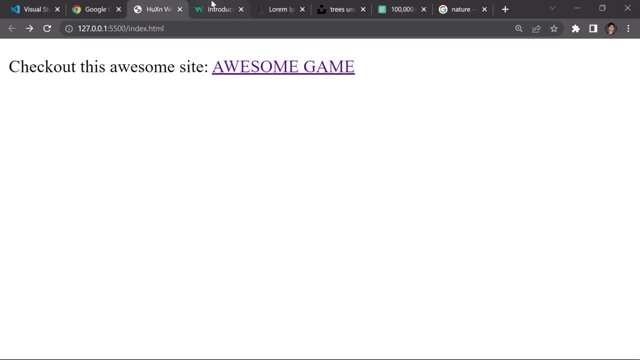 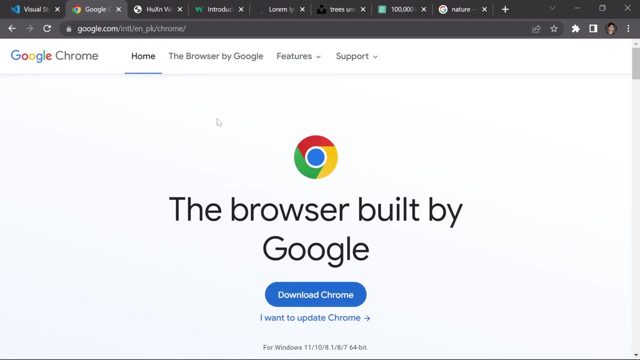 allows us to link to our own site, like in some situation. let me just go to this one, or, you know, let me just go in here here. you can see we are now inside this google chrome home page right here, but let's just pretend like this is your own website right here and if you just click on, maybe 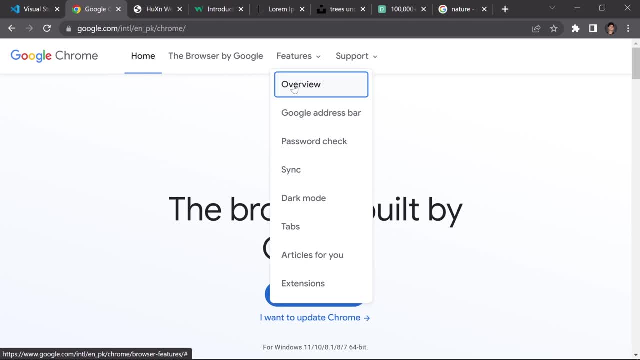 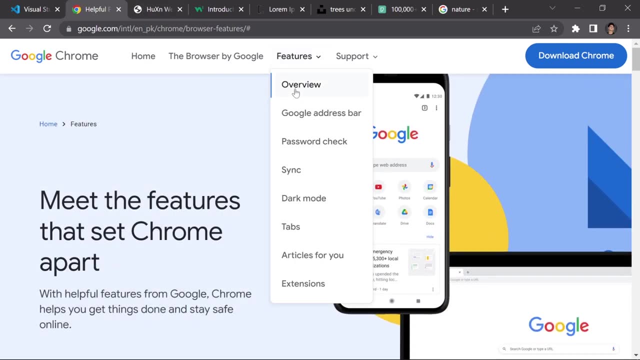 this feature one and if you want to go to the overview, so if you just click on that, it will now brings us to this overview section right here. so this is our own site and now they are known as a hyperlinks. the syntax will be totally the same, but they are known as hyperlinks, link that to some. 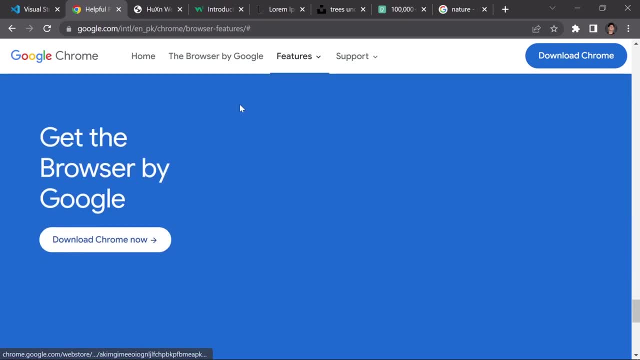 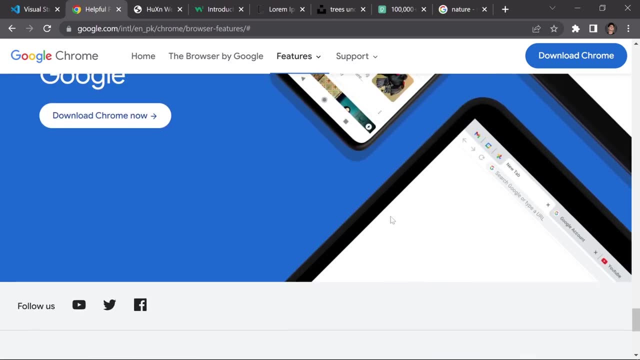 sort of other website on the internet, like in some cases we will just get to see, maybe a chromebook. these are all about a chrome, but i guess they didn't provide any other links to other pupils, but maybe, uh. okay, here you can see. we can now just click on this person. 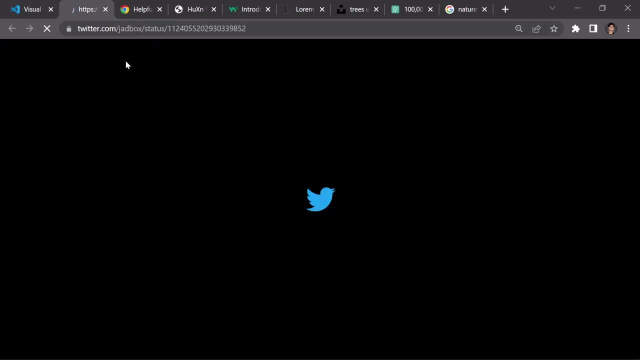 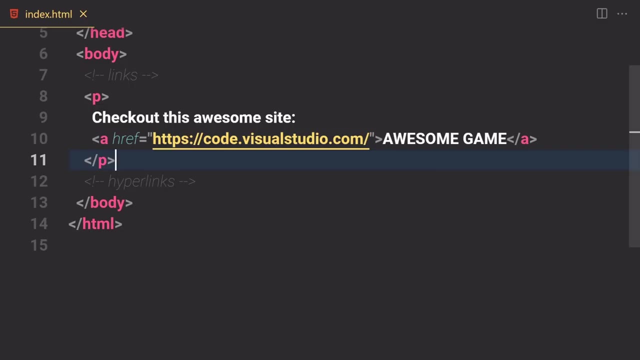 a profile and if you click on that and it will now brings us to another kind of a twitter website right here. so this is now known as a link, and i'm going to also ask from a google like: what is a difference between links and hyperlinks? but before we do that, i'm going to remove this coding from. 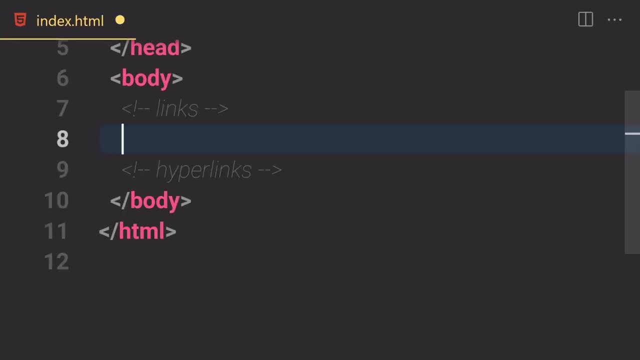 here and i'm going to zoom in a bit so you guys can see everything a bit better. and now i'm going to zoom in a bit so you guys can see everything a bit better. and now, if you want to link to some sort of other site on the internet, so for that we can just write like first of all a, not just uppercase. 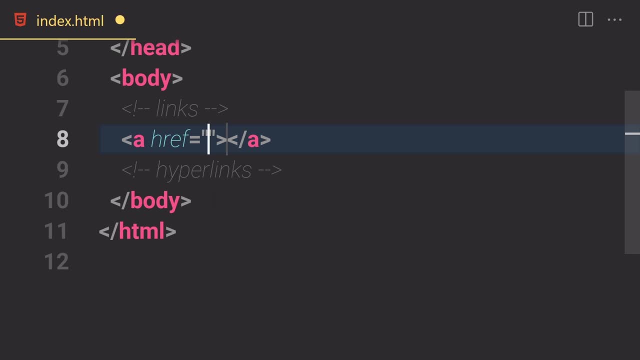 but a lowercase a, and if you hit tab- so here you can see- it will now give us like a opening tag and then a closing tag, and then it will give us this href attribute and here we are going to be placing the link uh, where we want to redirect our users. but first of all let me just write, maybe 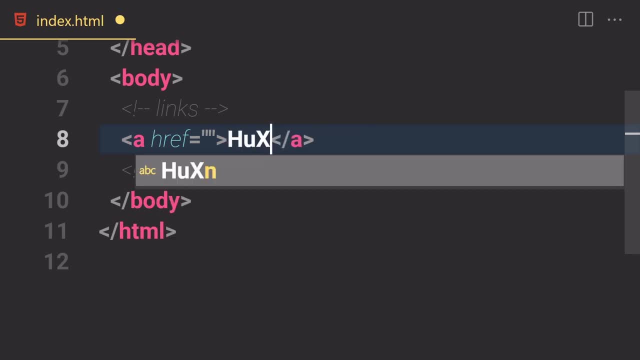 uh, some sort of a label for myself, like in my case, i'm going to just write like huzzain- yeah, huzzain would be good, be fine. and if it's our file- and here you can see the log- uses this link right here. so if you just, 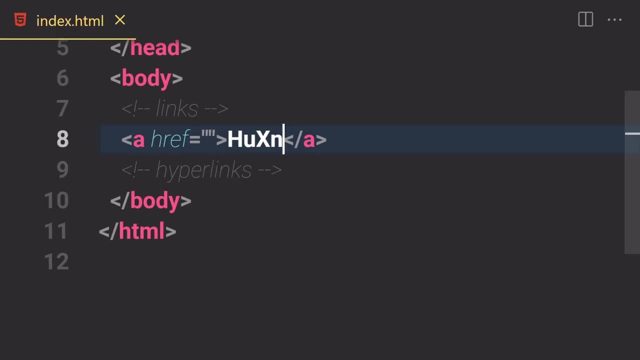 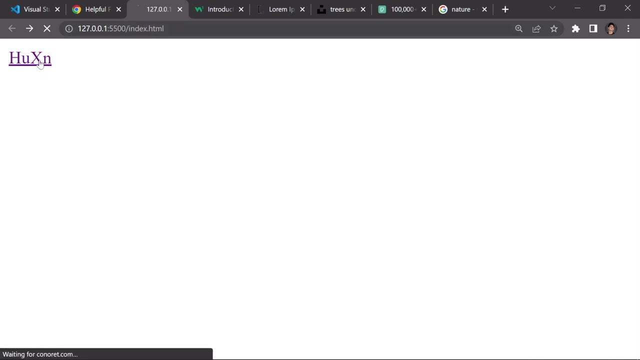 click on there so nothing is happening, because we didn't provide anything inside this href attribute. so that's why it's just refreshing our site, like i want you to just notice this area here. you can see, like anytime i click on that so it will just refresh our web browser right here. okay, so we can. 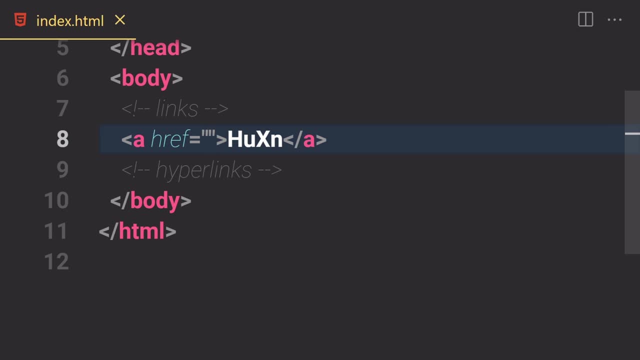 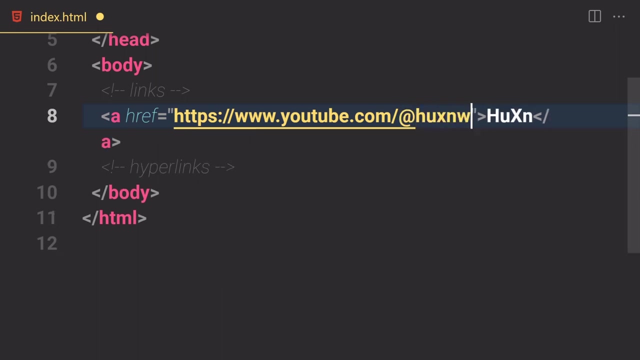 specify the link. if you have one now let me just write like: https: i'm going to link it to my own youtube channel. so wwwyoutubecom forward slash. i'm going to zoom out of it and then let me just write this: ad symbol and huzzain. 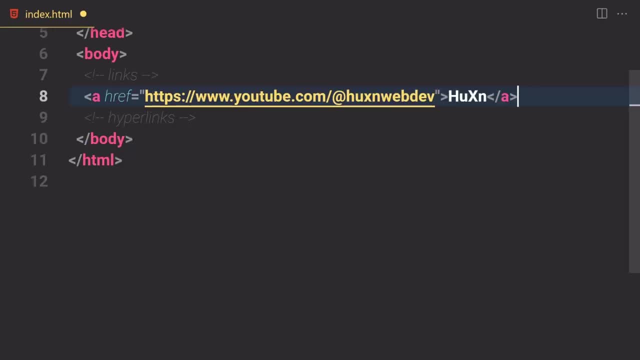 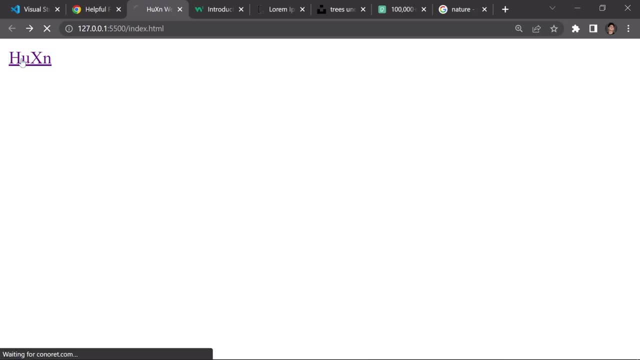 web dev and i just got this level, uh, a few days ago, and you also check out my subscriber in a second and i'm gonna save this file. and now, if i just click on this, huzzain and it will brings us to my own youtube channel right here and congratulations, we have 887. 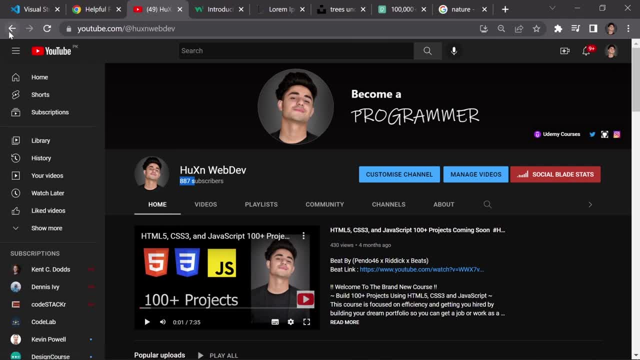 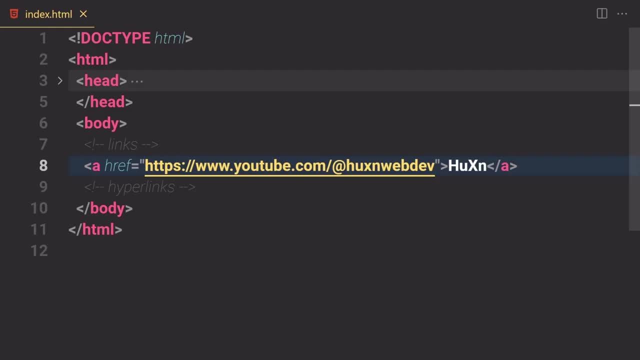 link that to our- not our own- web pages, but to those pages which are available on the internet somewhere. so we can just remove that and we can also remove this huzzain and we can just place like: maybe twitter for this case. we can also link that to twitter if you want to. so you can just 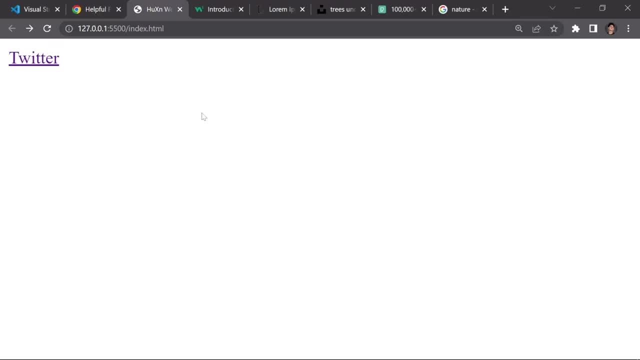 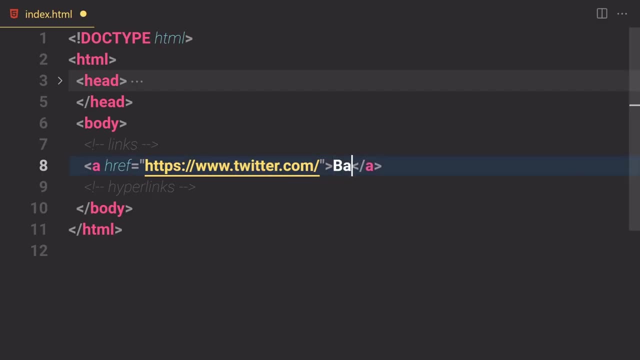 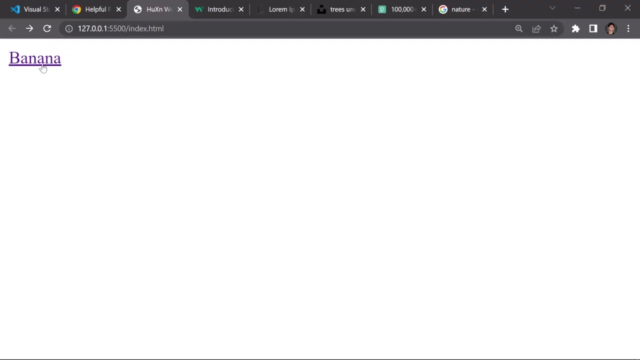 write like twitter instead. so if you save our file and now here you can see it no longer uses twitter, that's because we provide a label to be twitter. we can also write bananacom and it will still brings us to that twitter because, uh, as the link, we provide a link to be this trader. okay, so if you just click on this bananacom, 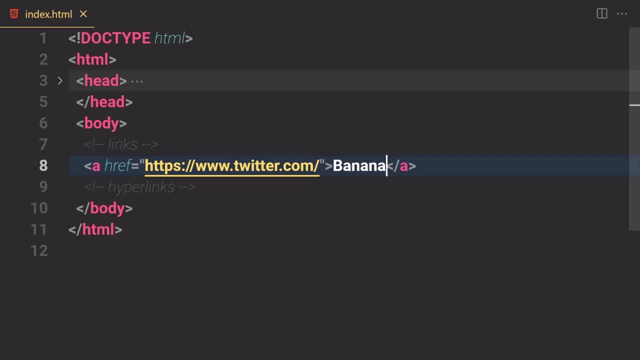 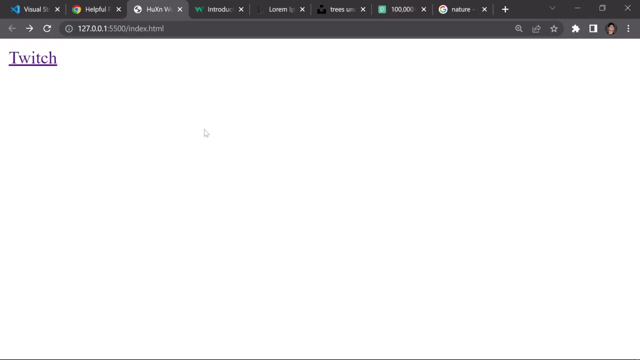 so it will now still brings us to this uh, twitter right here, and that's kind of a thing. maybe just change this one to which dot tv, or you know what. i'm gonna just write twitch right here and let me just write twtch for a twitch, and then here, dot tv. and if we save that, and now, if you just right click, 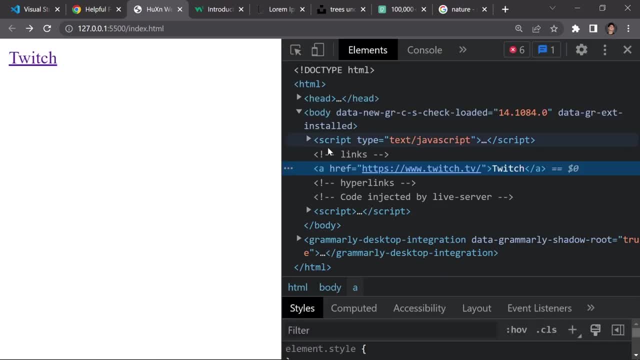 on it and then if you click on this inspect area, so here you can also see like. so in some situation you are not going to see that you can also see like. in some situation you are not going to see the link, and then you can just right click on it and then check it out inside our developer tools. 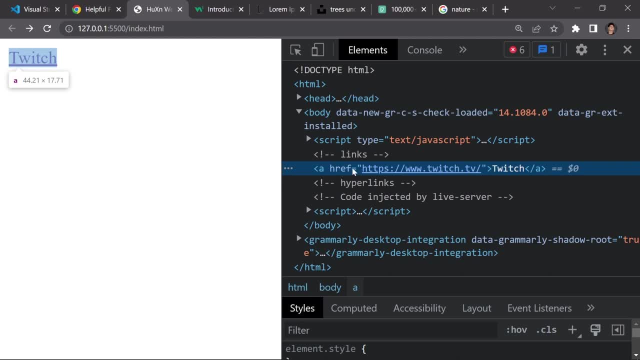 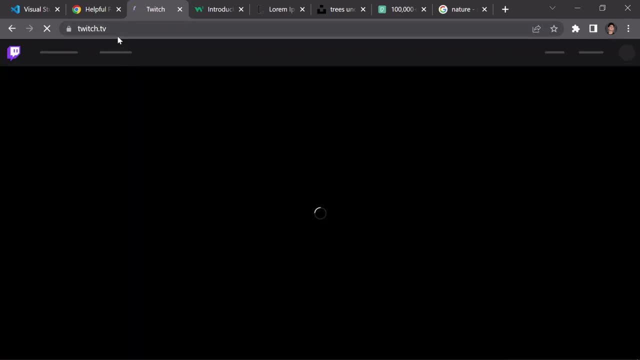 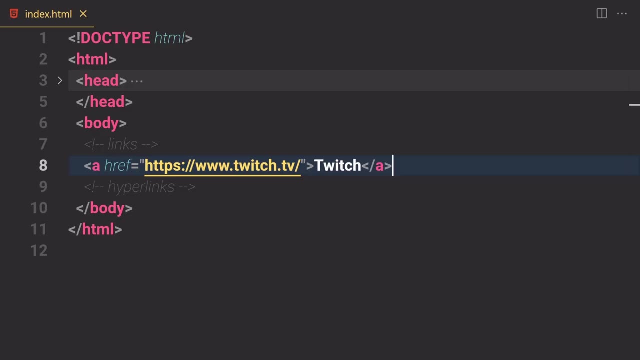 like here. you can see we have this anchor tag, then we have a href attribute and it goes to this twitchtv. okay, so let me just click on that and it will now brings us to a twitchtv website right here and it's awesome website. to waste your time, so go back. i'm going to go back right here and 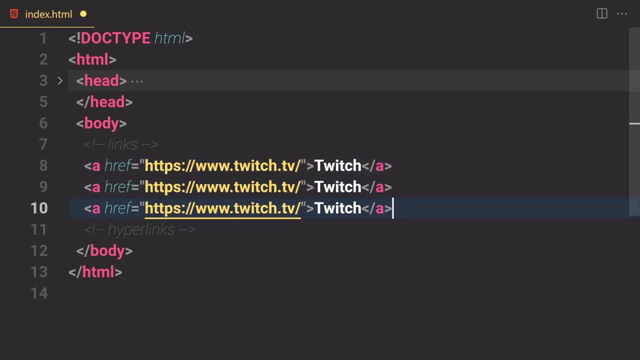 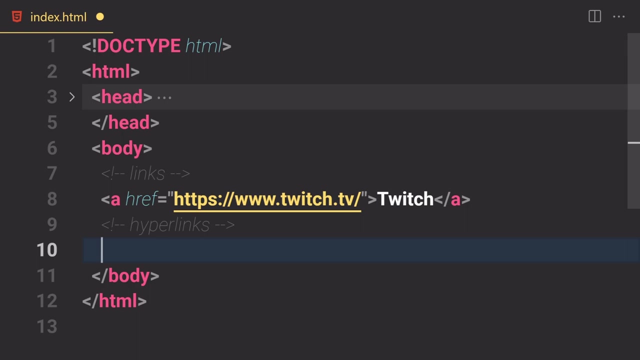 this is how we can link it to other website. you can like write more than that if you want to save it, and this is how it looks like: and boom. okay. so these are it about for links. so now let's just talk about our hyperlinks. a hyperlink will allows us to link through our own web pages, which 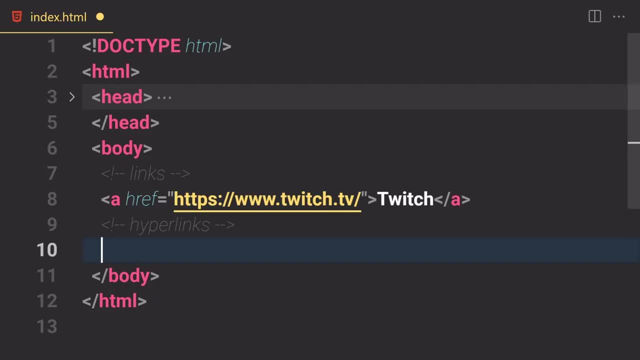 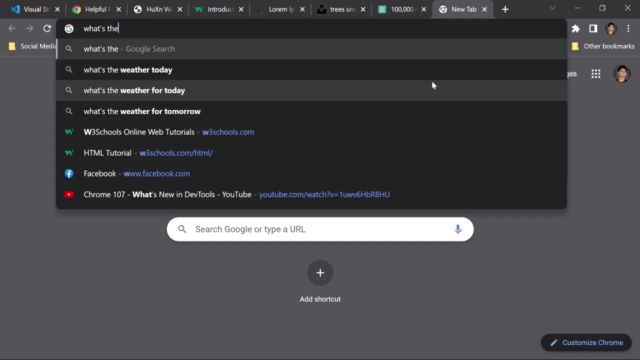 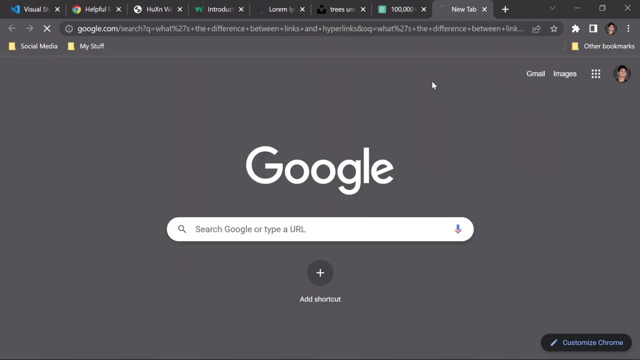 are currently available inside our own website. okay, so i'm going to remove that. and now let's just ask from a google like: what's, what's the difference between- uh, i don't know, uh- links and hyperlinks. okay, so google will help us all, right? so the main difference between a link and a hyperlink: 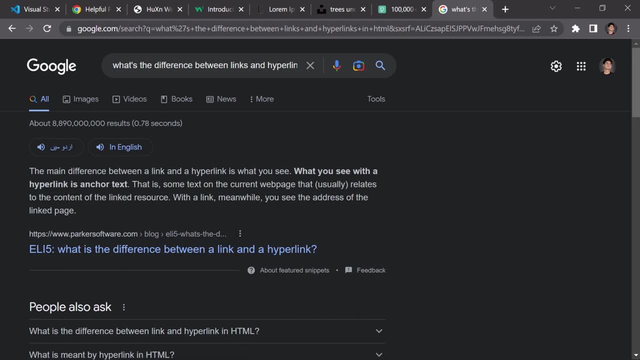 is that what you see with a hyperlink is an anchor tag text, that is, some text on a current web page right here that usually related to the content of the linked resources with a link, while you can see the address of the link. web pages like those link, which will brings us to, or redirects us to, some 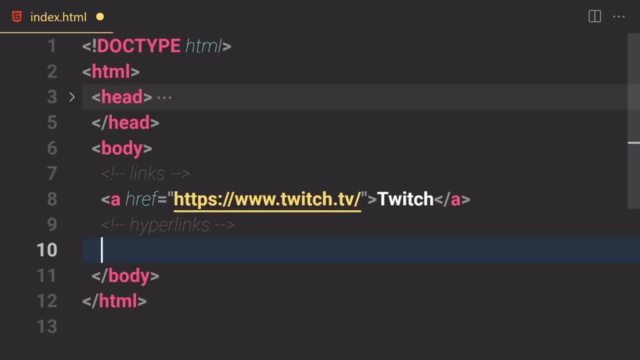 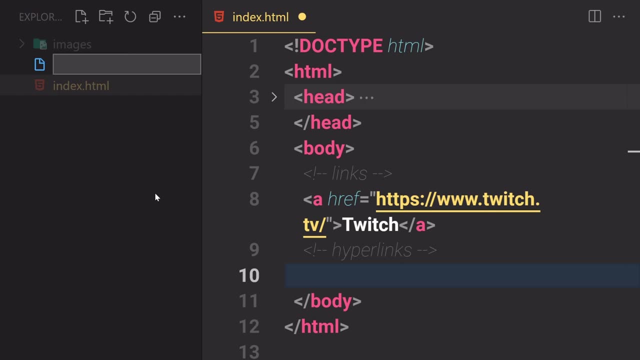 other web page on the internet. okay, so that was the main difference. so now let me just create a new file so that we can link through there. so we just have to click this new file icon right here and then we have to specify some sort of a name, or we have to give some sort of a name, not specify. 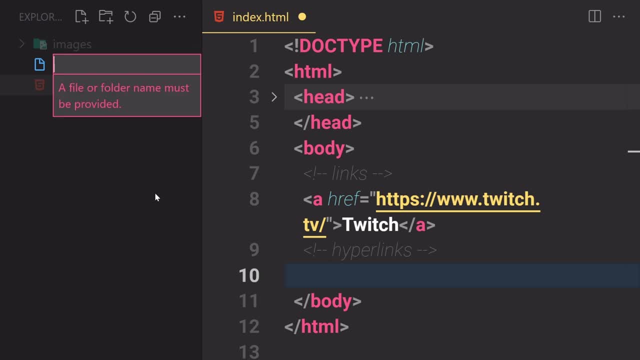 and now let me just give a name of like i don't know, banana, or you know what, orange- nah, i'm not orange and bananas, but i'm going to just write like another uh page. yeah. or you know, i'm going to provide like about dot html. remember, this first name doesn't matter, but you have to provide this. 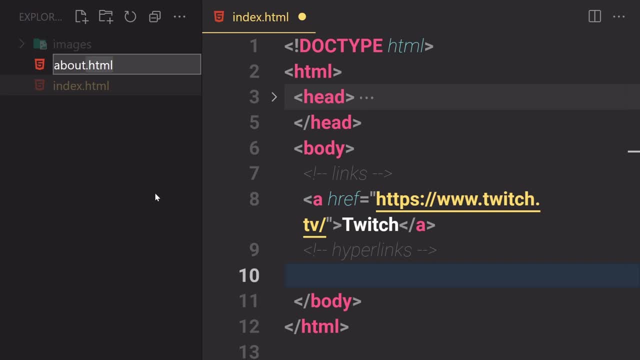 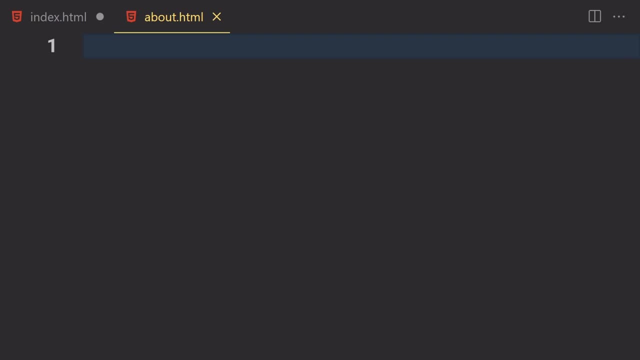 dot html extension, because this is important. so if you want to provide this extension, you have to just hit enter. so we'll now just create or about section for us, i mean like about web page for us. okay, so now if you want to get uh html code really quickly in a second, so for that you just have to. 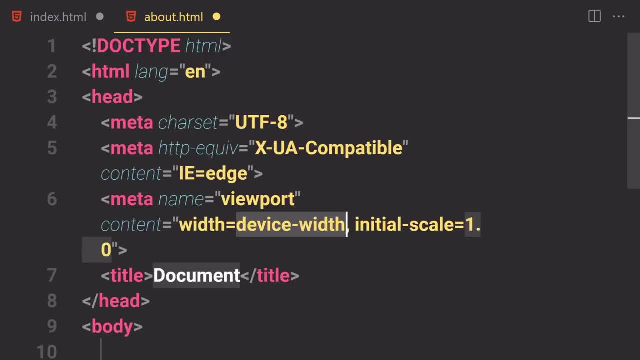 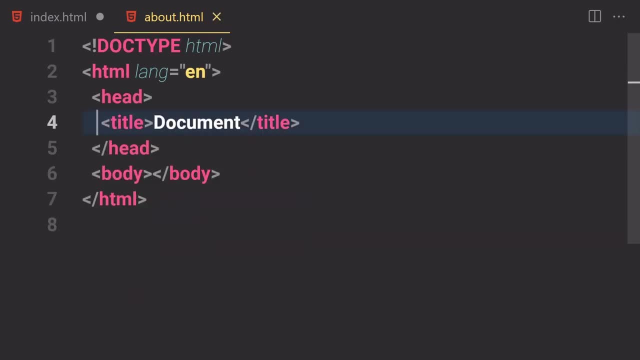 write this explanation mark and then i want you to just hit tab. so here you can see: unlock uses the html structure right here. so what we have to do, i'm going to remove all of these metadata's from there, and that is something called uh emit, which i just used in a second, and we are going to be. 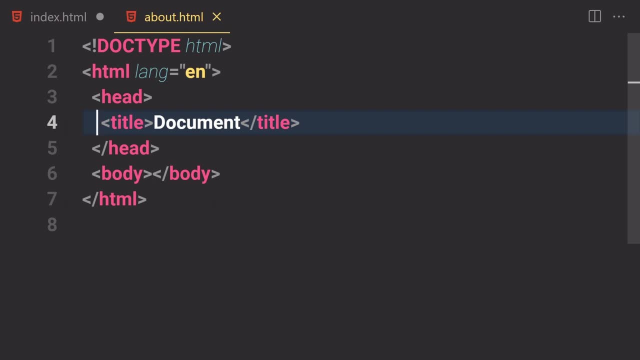 learning about a crazy image later on in this video. so let's get started, and let's get started with this code, start with the h1, but here we're just going to check out this h1 where and anyway in this page, uh, pmd is allowed, that it also has a ICT and thus tumbler possibilities it provides. 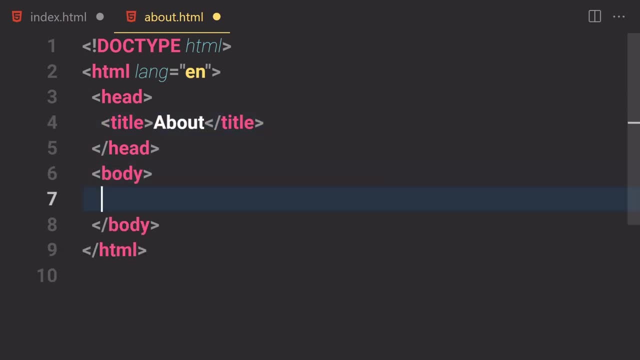 us a lot of the damny editing features for material and trying things to open up like i أي about section or you know you about, will be just fine. so i'm going to just stick with this about and here we're going to just write in like h1 of: uh, welcome to the new page. okay, so if we 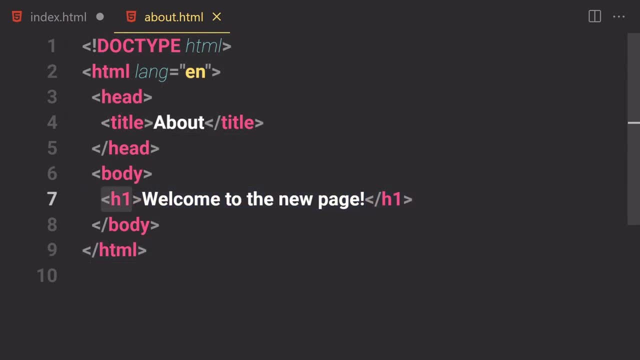 save that and now we successfully create our indexline html file. we just put all of our content, or welcome, to the new page. now what do we have to do? we have to link this uh web page to this indexhtml file. so how can we do that? well, we just have to write this anchor tag and if you hit tab. 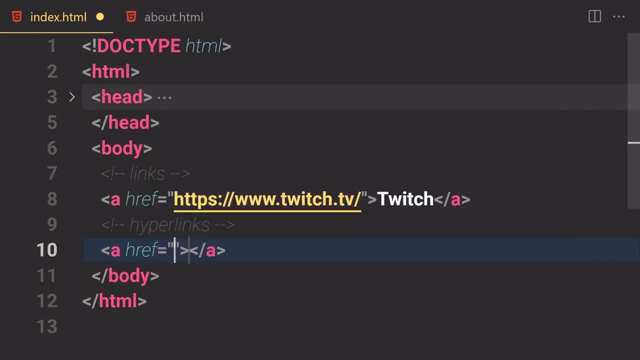 so it will now give us this href right here and all of these stuff. so if you hit control and space, so it will now gives us everything which are currently available inside our directory. so we are going to be selecting our abouthtml file and now here we are going to be just writing. 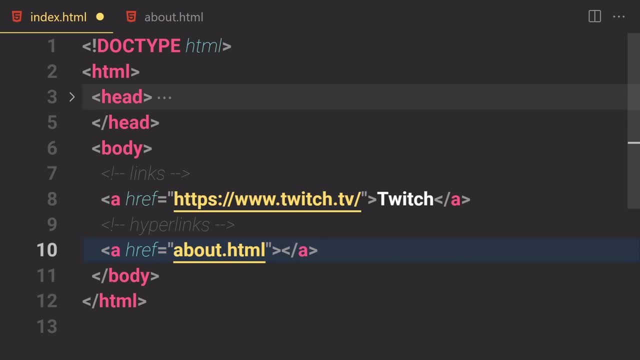 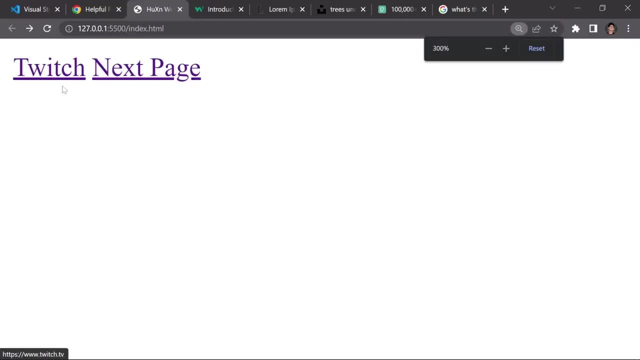 a label of like anything. you can write anything if you want to, but in my case i'm going to be just writing like next page right here and if you save that, okay. so here you can see, we have this twitchtv. this is a link and now this is a hyperlink. so if you just click on that and boom. so 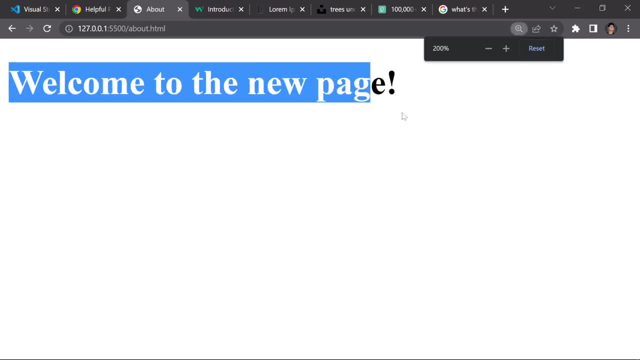 what do we get? we get like: welcome to the new uh page right here. okay, so this is how we can link through by using our html. so if you go back and here, i want you to also notice this uh url right here. so we have this indexhtml file right here and we have this indexhtml file right here and 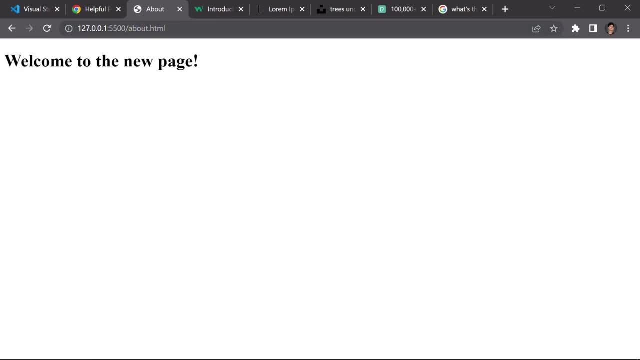 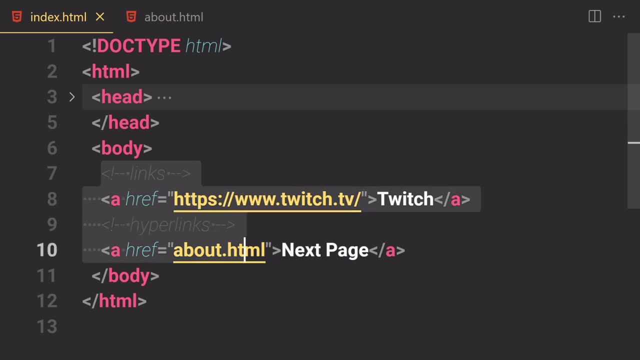 if you click on this next page, so it now brings us to this abouthtml url right here. okay, so this is how we can work with the links and hyperlinks in html, so i'm going to just remove that now. the next topic which we are going to be learning about is something called 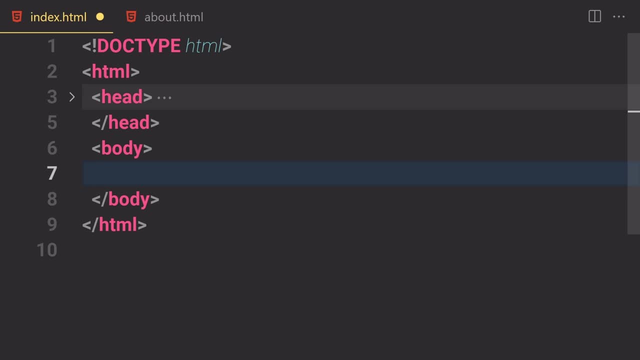 uh, forms and inputs, and it's kind of a little bit huge topic to learn, not a hard one, to be precise, but a little bit long, like we have a lot of input tags and stuff like that. so get ready. so i'm going to just save this file and here you can. 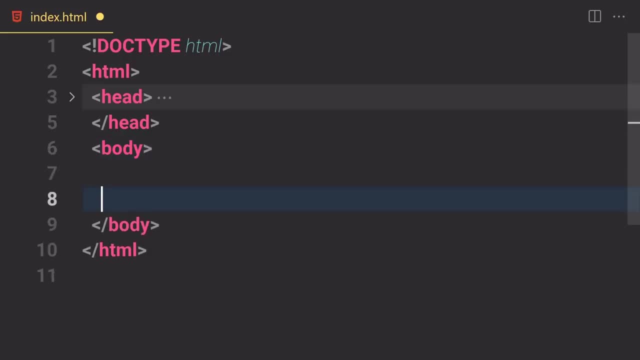 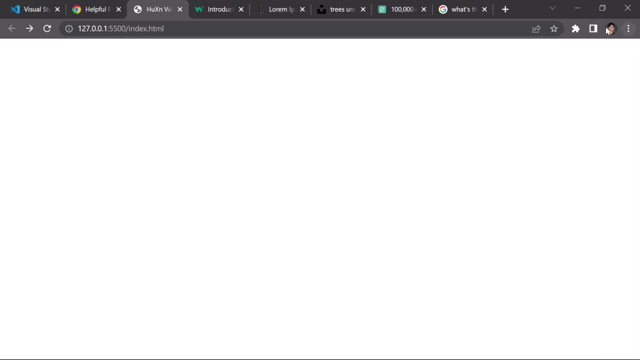 see, we don't have anything inside this body tag. so now, in some cases, you just want to work with the forms like: uh, i don't know, let me just create. let me just launch a new tab which is known as incognity. so i'm going to just click on these three dots and then i'm going to click on this. 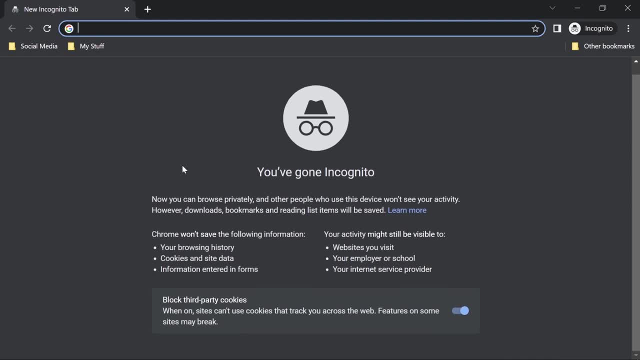 new incognity window so you can learn more about this incognity window if you want to, but basically incognitive window. don't have any kind of a history tab or right here, uh, this, uh basic one do have this history tab, which is right here, but 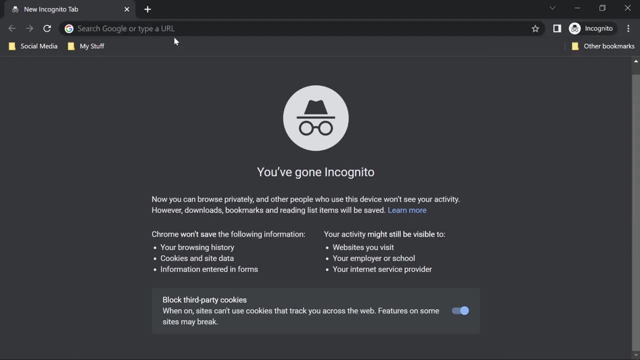 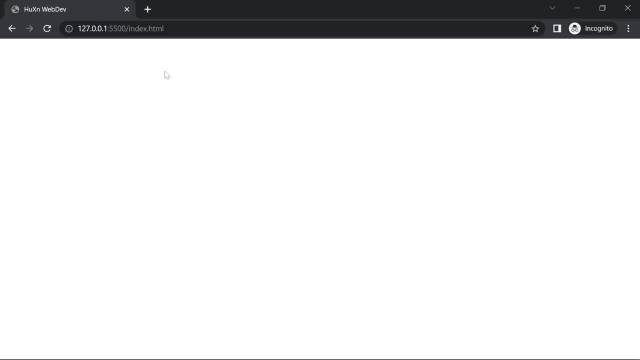 this incognity- will not have that history tag, so you can just search anonymously if you want to. so what i'm going to do, i'm going to copy this url from here and i'm going to paste it right here. i mean here, if you just click on that. oh, you know what we're not going to be doing? that we have to. 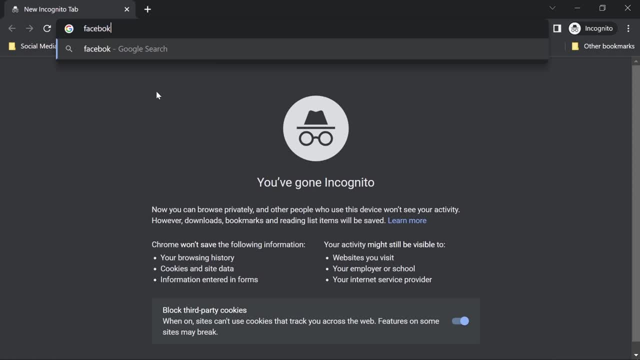 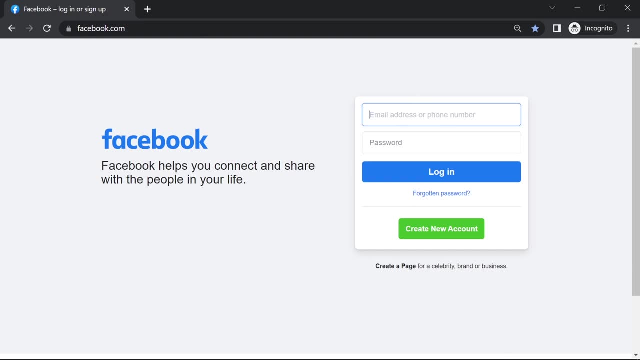 just write like: maybe facebook, uh, facebook, okay, dot com. and if you go to facebookcom and here you have this form right here, so we have email address or phone number, and then we have a pencil right here and we have a login button and this kind of stuff, so we have this form right here. let me go to 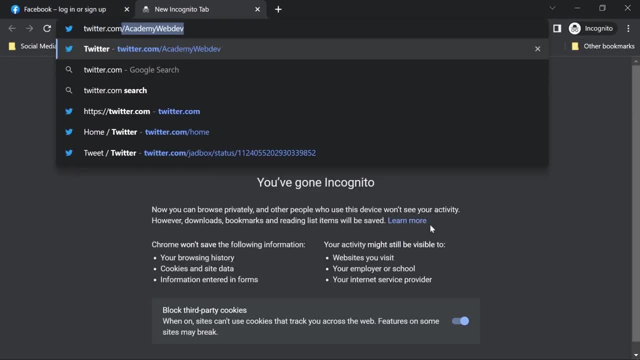 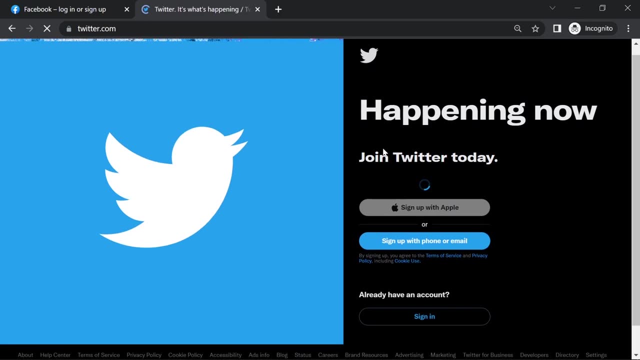 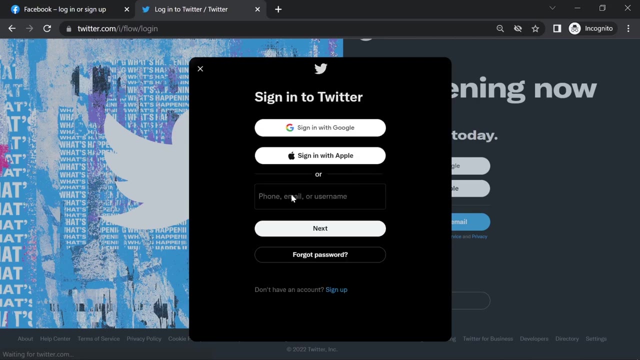 another website which is, uh, twittercom. okay, and i'm gonna remove that my handle. so if you go to just twittercom, so it will also ask us to log in or sign up, and we don't have any forms in there, do we? if you click on the sign in button and now, here you can see, it now brings us this form. it's not a. 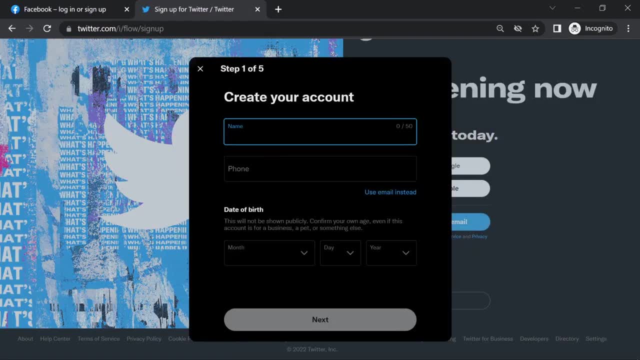 come on, sign it with your email or phone. so now it will give us like name and phone and then these kind of forms and it's tab right here. so what do i have to do? i'm going to just click on this x to remove that incognito window from now and now. here we are going to be building our first form. 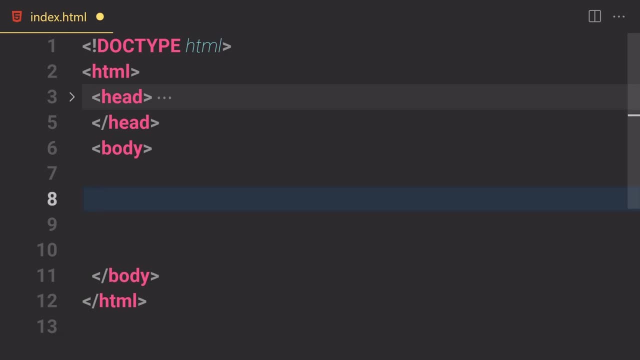 and we are not going to be sending our data to some sort of a server and stuff like that, because we are not working on a goal link and we are not using some sort of other bacon development right now, but we have to just create the uu or the user interface of our form. so if you want to do that, so what do we have to do? first of all, 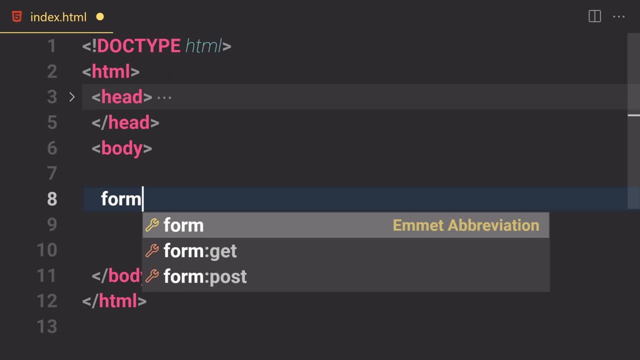 we are going to be just writing like f o r m, and if we hit tab, so it will now give us form opening tag and form closing tag. so now, what do we have to do? i'm going to just remove this action for now, and this action will ask us like: where do you want to send your data we don't want to send. 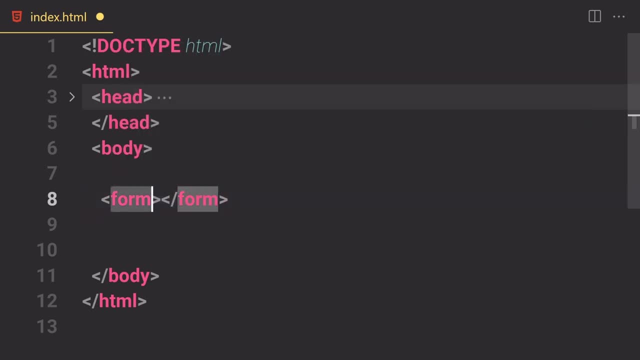 our data to anywhere. so for now, we just have form opening tag and then form closing tag. okay, so now, if you save that and nothing will happen right here inside our body now, inside this form, what do we have to do? first of all, we just have to write our label for the form. so let me just write l l a. 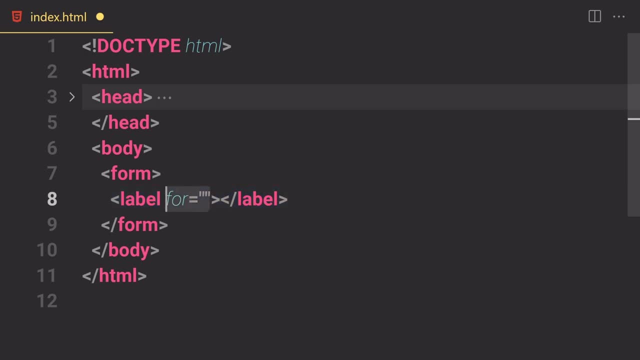 b e l, and if you hit tab- and we are going to be removing this for for now, and i'm going to also show you what is that for will do for us- but for now we just have our label opening tag and label closing tag. so here, what do we have to do? i can write anything i want, but we can just write our. 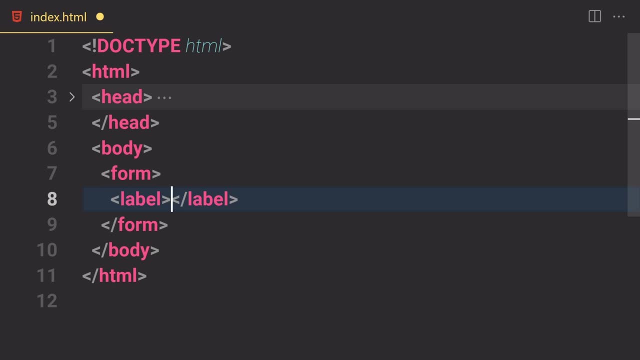 specific label like: maybe please enter your email. like: please enter your email address. oh, you know what, i'm not going to go that much crazy, but i'm going to just write like an email in here and if we save that and here you can see, we are now getting this email right here, just an email text, nothing else. so 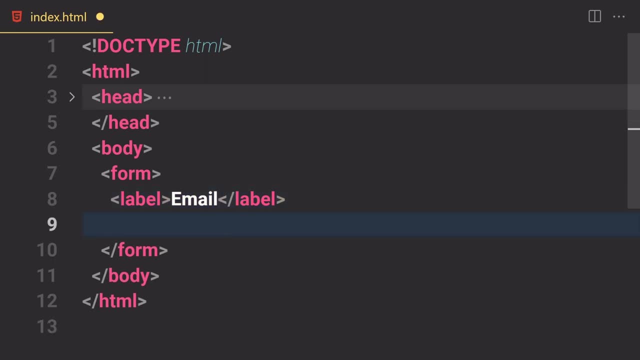 now, if you hit control and enter, so now we have to create our first input box. so if you want to create an input, first of all we just have to write i n p u t and if you hit tab, so it will now give us this in. and, by the way, this: 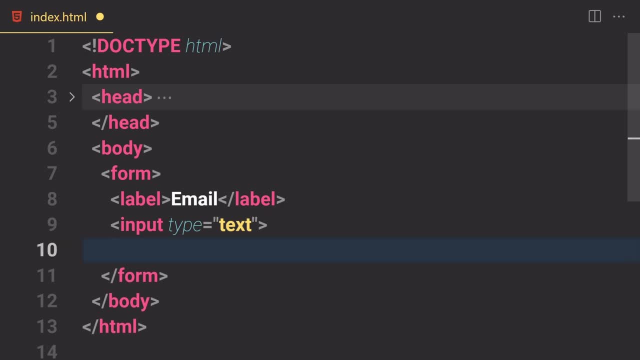 is a self-closing tag and we already learned about a self-closing tag, but i forgot to mention like img is also a self-closing tag. if you want to close it, so you can just write a slash in here, and this is also a self-closing tag in html, and this input is also a self-closing tag in html. so 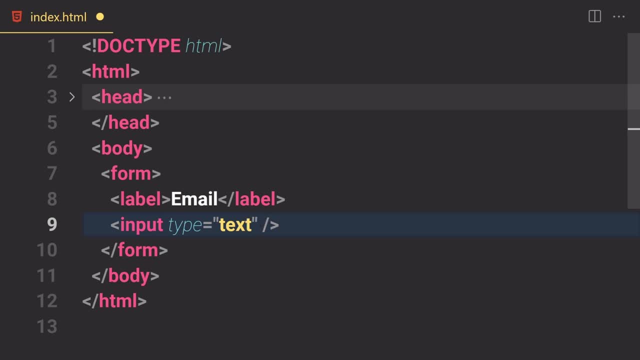 i'm going to just write a slash in here and now. here you can see, we have this type of text and we have a lot of types. so for now i just want you to write input and then hit tab, so it will now give you this type of text. so if you save this file, 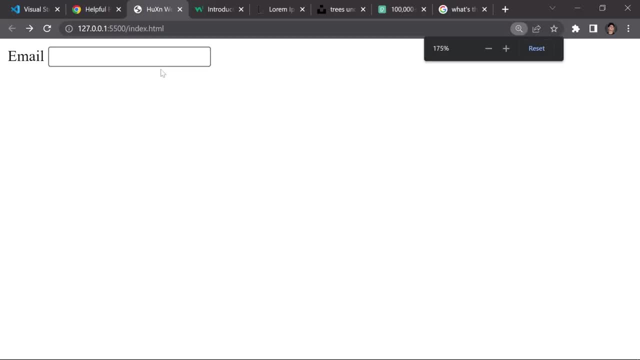 and boom. here you can see we are now getting this input area and we can type anything we want inside there. so we are now getting our email as a label and then we are getting our input area right here. okay, so if you want to break, so, in some cases you need a break from this email. so what do you? 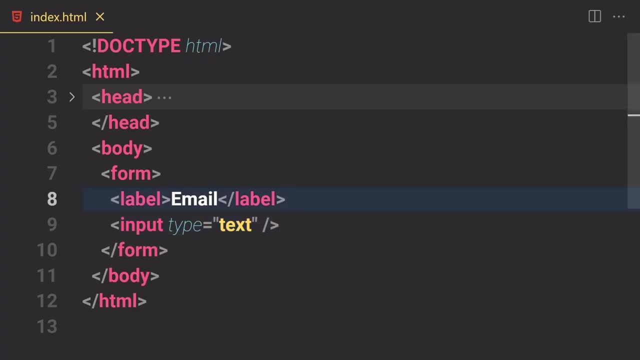 have to do for that? we can just write a special uh tag, which is also a self-closing tag, which is known as a br. if you just write a br and it will allows us to break the email and then we can type through this line. so if you save that and boom, here you can see, it will now just break this line. 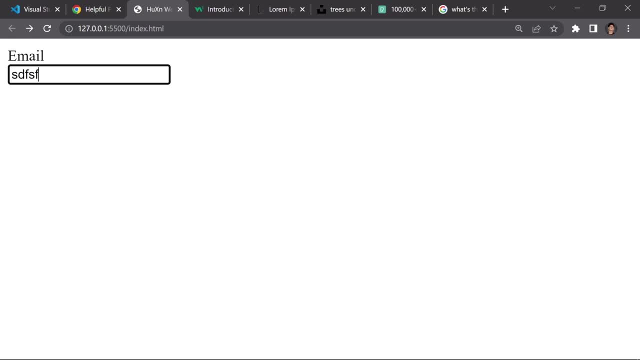 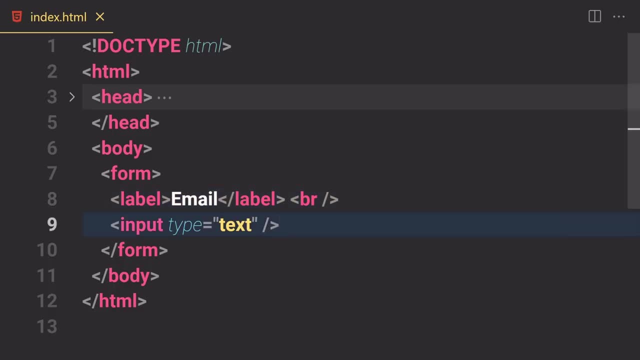 from here and we'll now just put this input area in a new tab right here. not a new tab, new line. okay, so this is our first email one. now, let's suppose if you want to create for something else, so if you just write l-a-b-e-l for a label, so why are we getting this for attribute like? so what is? 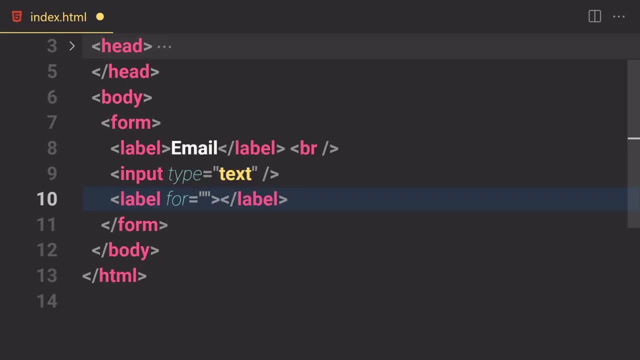 the meaning of this for attribute. let me just show you that. so here, in this case, i'm going to just put maybe, um, i don't know, i'm going to just put this for a label, and then i'm going to just put this for a label, i don't know. so that was an email, you know, i'm going to replace that to a name. 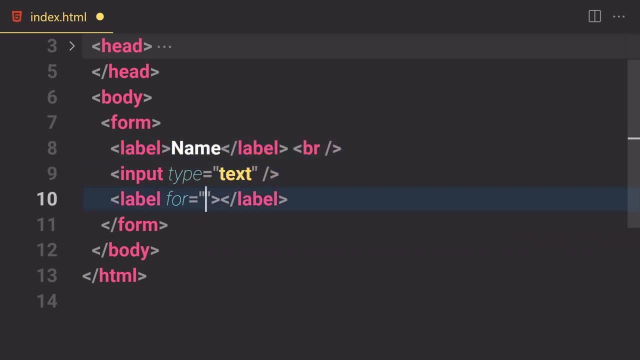 so this one will be a name and this one will be email. so i'm going to just put like an email in here, a lowercase email, and then the camel case e and then m-a-i-l, and i'm going to also just write an input right here and now, if i save my file. and now here you can see we are now getting. 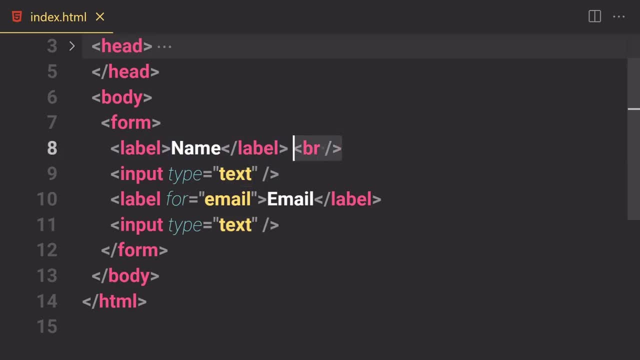 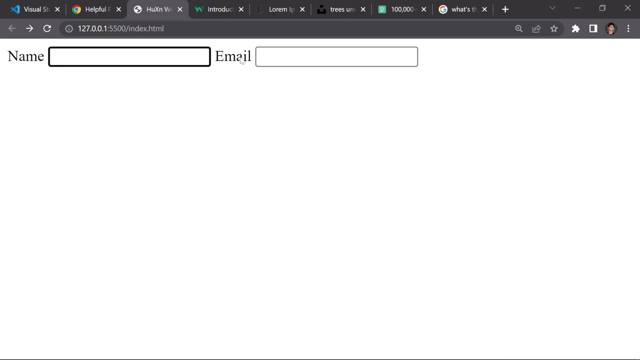 like name and then email. if you want to break and you know what- we are not going to be providing any breaks and whatnot- i'm going to remove this break from here and if you save that, we have our email. i mean, like we have our name and then we have our email, okay, so i'm going to also change the type to be email as well, and 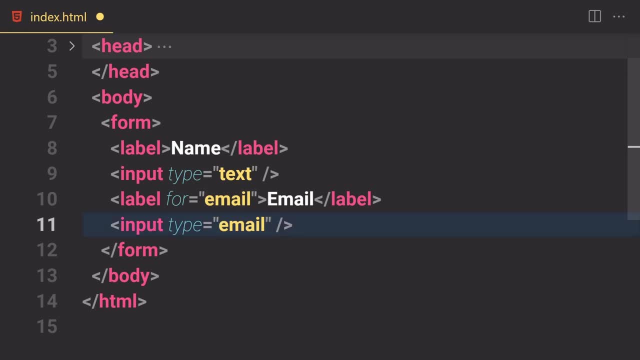 i'm going to also tell you why did we change that? but now that we provide a for attribute in here, so what do we have to do? we also have to provide id to it, id attribute. and here we just also have to type everything like anything. we write inside this for attribute. and if i copy that and if i 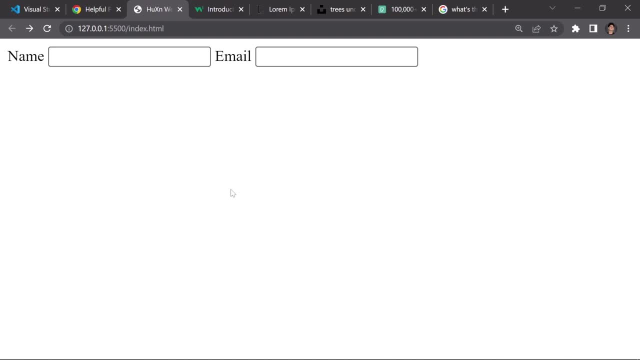 just place it right here and if you save that, so it will not do a magic for us. but if you click on this email, so here you can see- it will now just activate this input area for us right here. okay, in this case we didn't provide any for attribute here, but if you just click on that, nothing will. 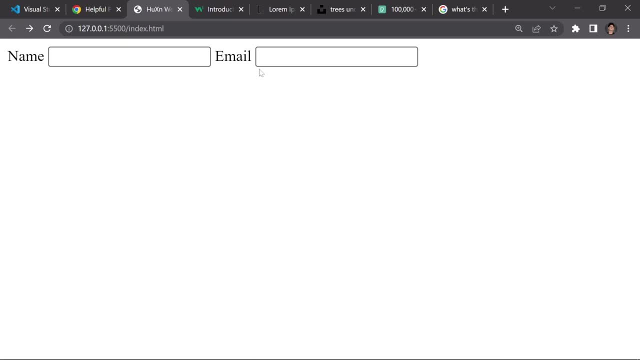 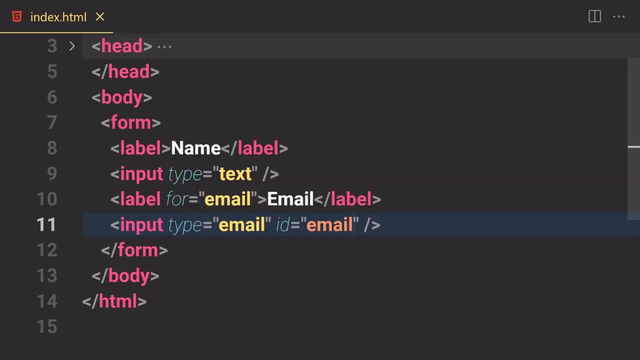 happen. if you click it one more time, nothing will happen. and if you click on this email right now, so it will activate or input area right here. so that's because of this for attribute. so anytime you want to activate by clicking on this email so you can just type like um, you can just specify. 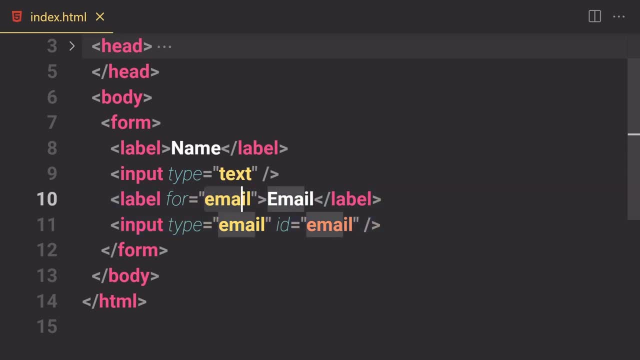 this for attribute to it and anything you write in here. you can just type in here and you can just see it will start up in this for attribute and you have to put that data inside this id as well. i know this stuff are kind of confusing and not giving us that much of results, but you don't have. 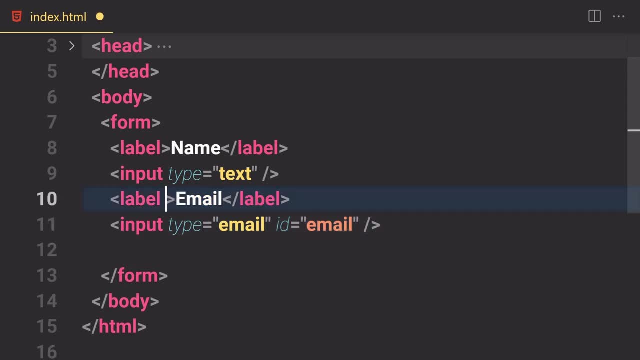 to worry about that. if you just want to remove this, you can also just remove that from here, so that we can just work on our simpler code. so i just kind of want to show you that for attribute as well. so we are now done with a name email. so now let's just talk about a password one. so we 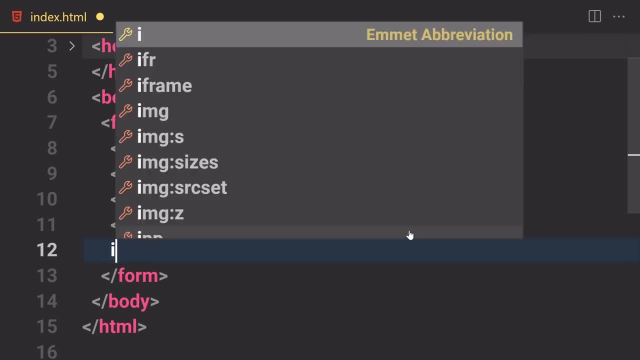 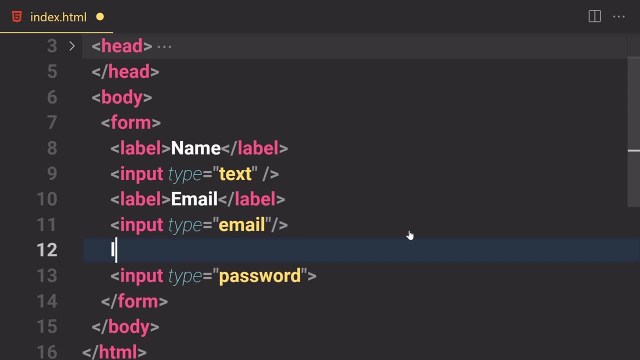 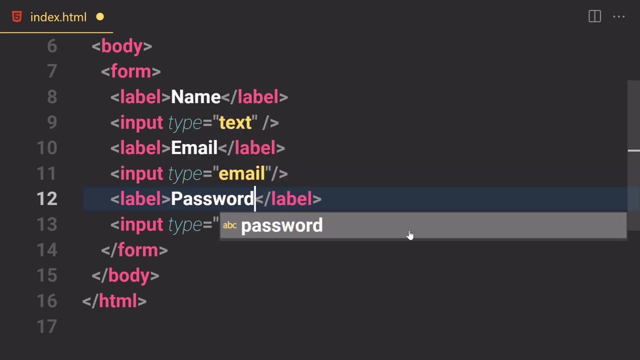 are going to be just writing like password, not password, but we are going to be just writing in: and now let's just change this text to be password. and we already forgot to include our label for here, so i'm going to just remove that for and here we just have to write our password. and now, if we 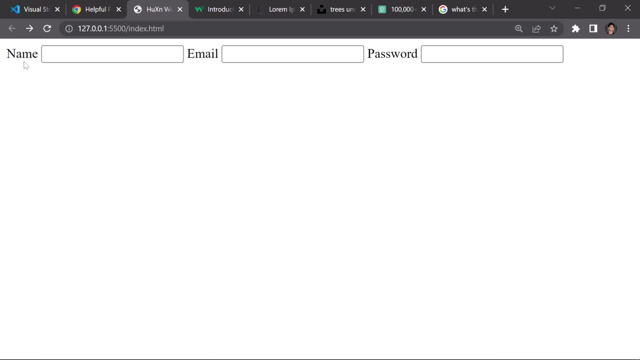 save that. i'm going to just zoom out of it. we have a name, then we have an email, then we have a password and anything i write inside this password input area will not show up to the user. so we can do one trick for that. so we just have to right click on it and then click on this inspect area. 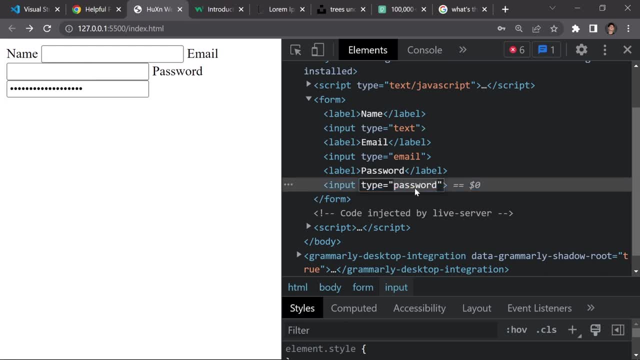 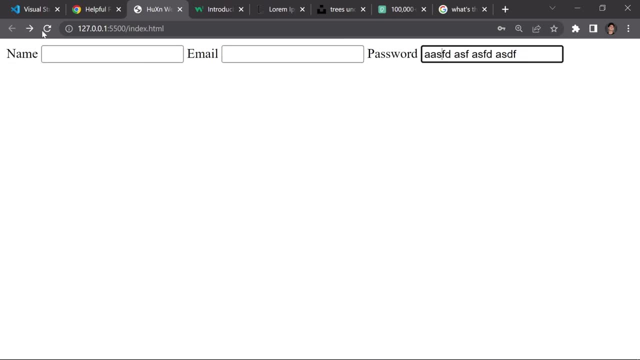 and now here, instead of writing a type to be like a password, we can change that to text and if we hit enter and we can see our password right here. but you don't have to do that. we can just refresh our browser and if you type something so it will not show up to the user. okay, so we learned about. 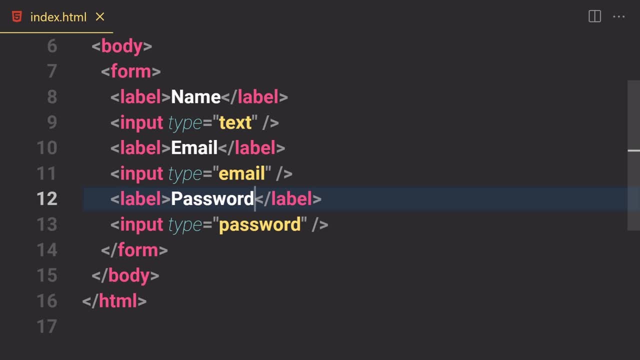 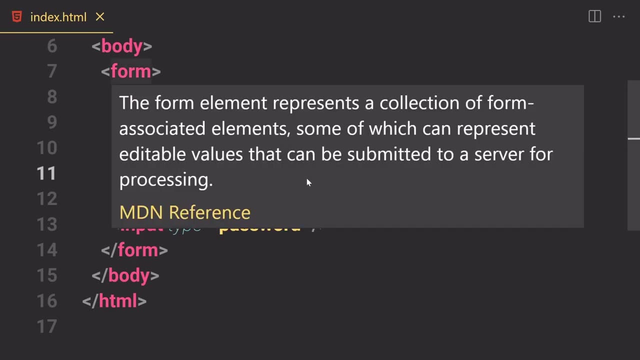 input of tags, input of email and also input off. and, by the way, i forgot to show you like: what will this email do for us if i just type something inside that? oh, first of all, let's just learn about the new one, then you can get to know what it is. 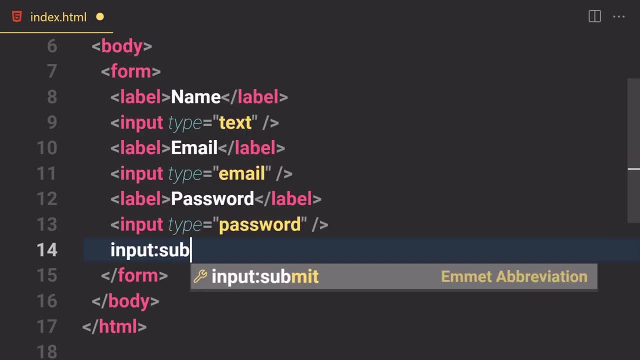 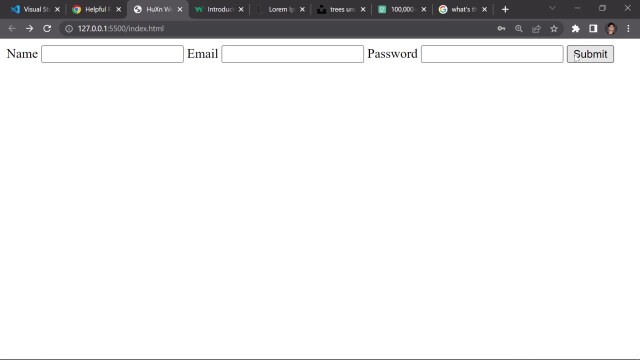 this email one, so we just have to write our input and then submit. okay, so the type will be submit, the value will be nothing. so if you save that- and here you can see, we are now getting this input of submit right here, so it allows us to submit our data or to just clear out these forms right here. 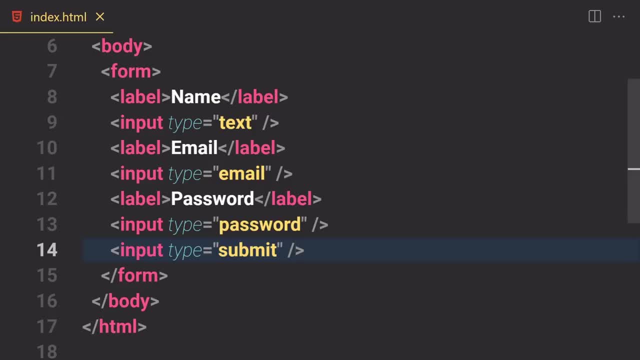 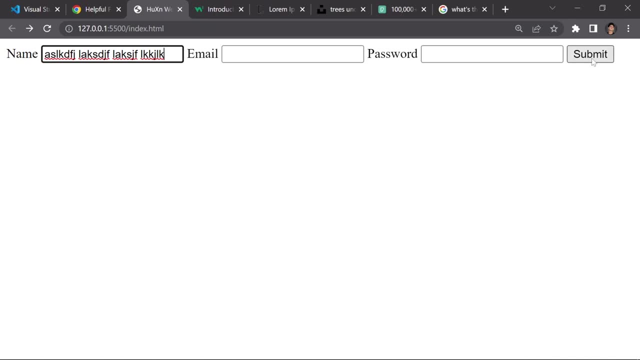 or to be precise, these input areas. so now let me just type something in here, like we can type anything we want inside there and it will not complain. so if you just click on there and boom here you can see it will now just send that data to nowhere. so it will just. 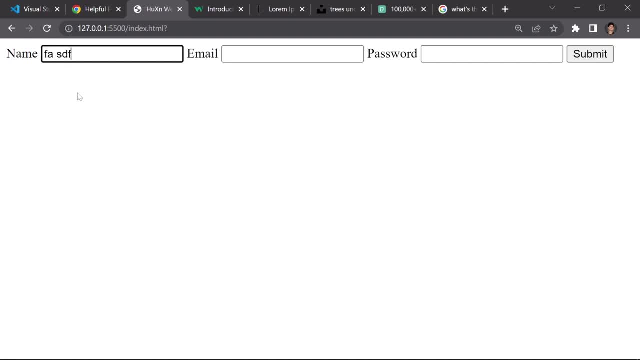 remove that data from inside this input area so we can type like anything, like a numbers or maybe assembles, like that. we are totally free. but in email, anything we write like, we have to provide a valid email right here. so it will require us this add symbol. so you know what i'm going to. 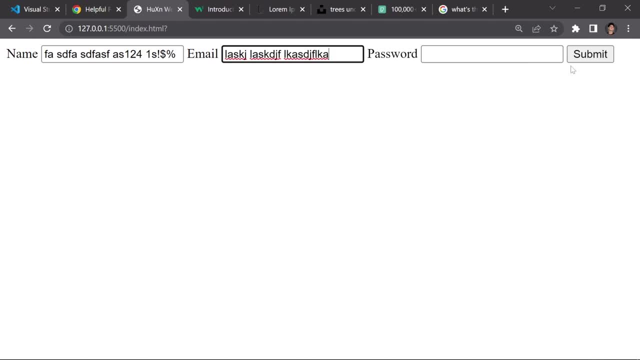 just type like this jibberish right here and if i try to submit my form, so here you can see it's asking for: please include this add symbol in the email address. you provide that and it requires us to do that. so here if i just type like, maybe test at the test or, you know, test at gmailcom. 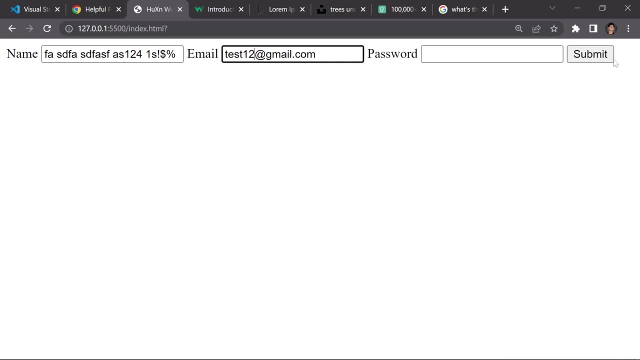 test at one, two, three or one, two would be fine. and now, if i try to submit that, and here you can see that data will be sent to nowhere and these- uh, here you can see- it will now just empty up all of our input areas right here. okay, so this is how, or we can work with a text email and a password one. 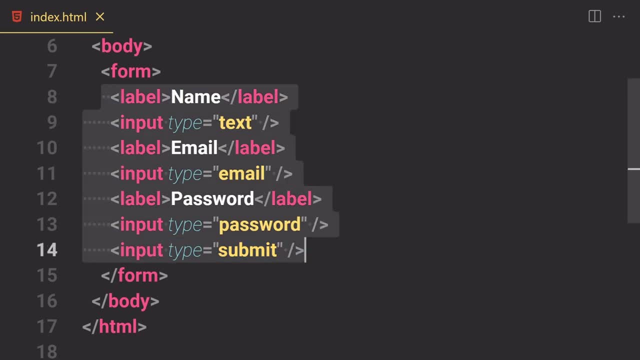 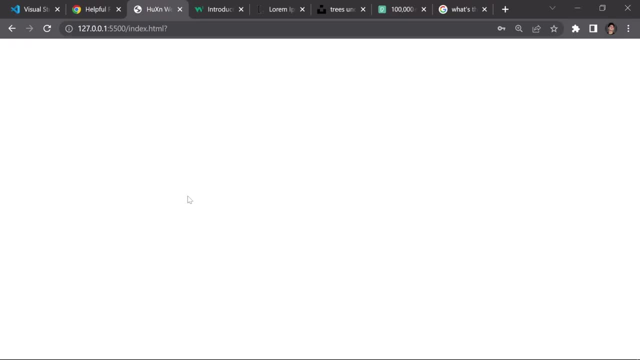 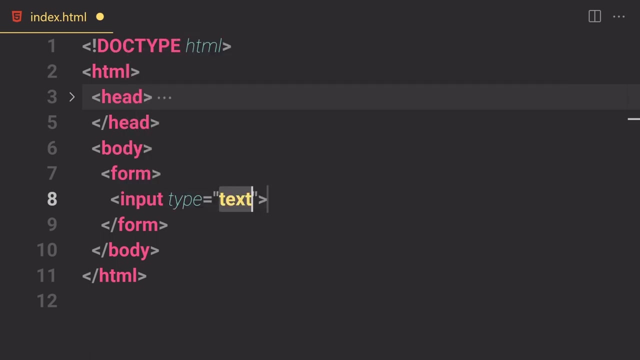 okay, you know what we learned. enough about labels and stuff. so what do we have to do? we have to remove all our text if we go to achievers and if we go to save and in here there, we have to remove almost all of these from here. so we have to remove one of these is not a form one, so we do have our. 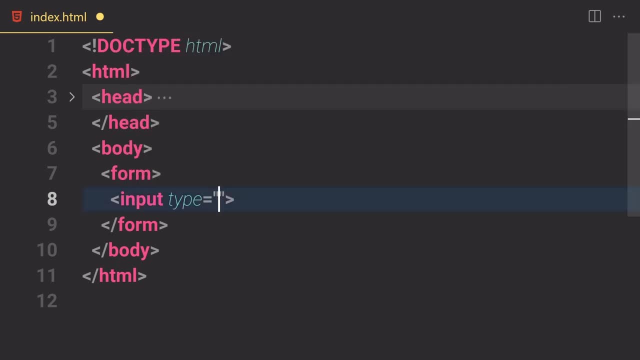 form right here. and if we save that and we cannot see something? so now let's just discuss that input areas one more time. so now, if i just type like input in here, so here you can, several log users, these tags right here, we can remove that. and if we just hold ctrl and if you hit space, several log. 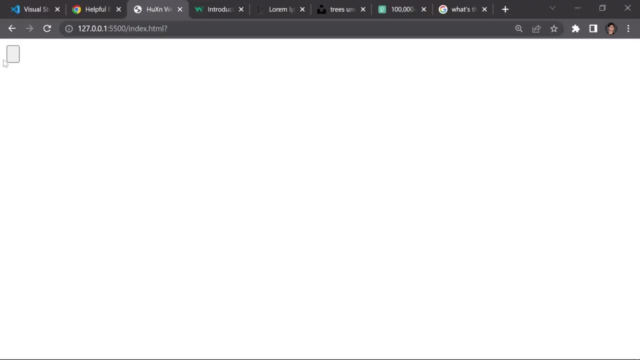 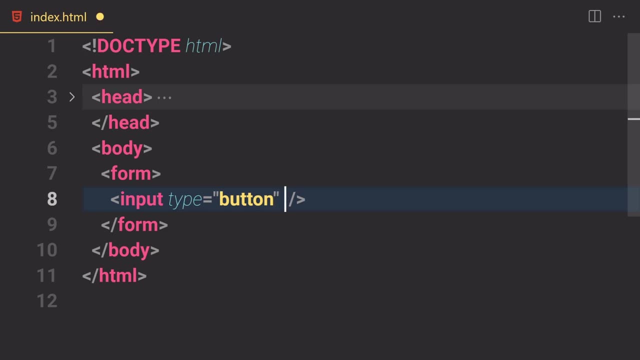 users a lot of input types right here. so we have button, we have checkbox and all of them. so let's there and here you can see it along. uses a button with no label and whatsoever. so if you want to provide a label for this button, so for that we can just write like a v a l u e, like a value attribute. 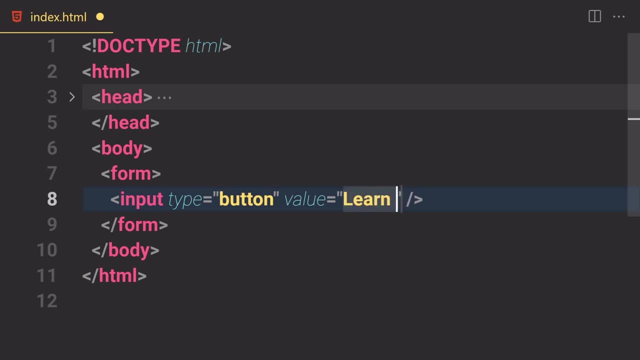 and we are going to just write like: maybe learn more, and if you save that, and it will not give us a label of learn more. we can also just write like: uh, maybe excuse me, you can also just write like a download, if you want to, and if you save that, and it will also give us that download and 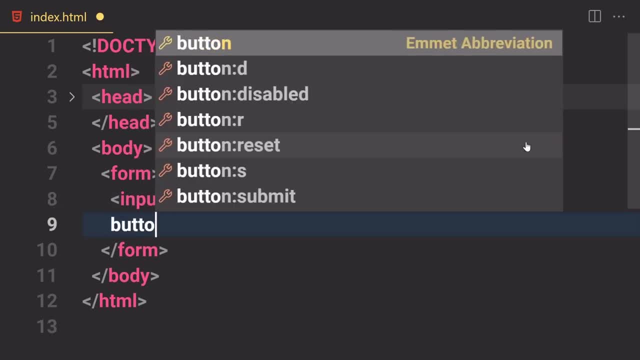 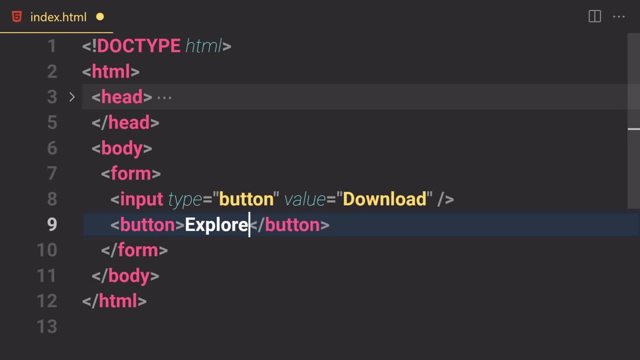 we can create our own buttons if you want to. so we just have to write like a button and we can just put our content inside there. maybe i just kind of want to write like explore, and if you save that, it will not use this button of explore. we can write: uh, explore the nature. we can type anything. 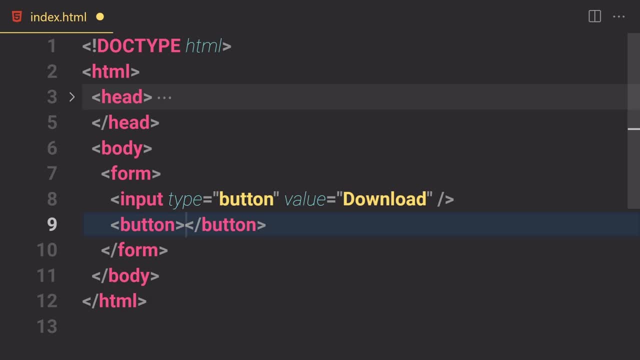 we want inside this button and it will still work. so in this case, what do we have to do? we just have to write like: maybe download, and if you save that, it will also gives us these same buttons right here, so we don't need these uh type of button. so i'm going to just remove this value from here, or you know what i'm going to. 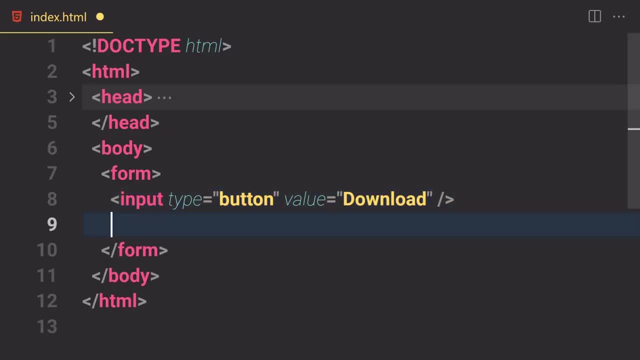 place it right now, just for demonstration purposes, anyways. so now let's just create our new input box. so i'm going to just write input and i'm going to remove this text from here and now. what do we have to do? we just have to hold ctrl and if you hit space, so we have our checkbox. so it will now. 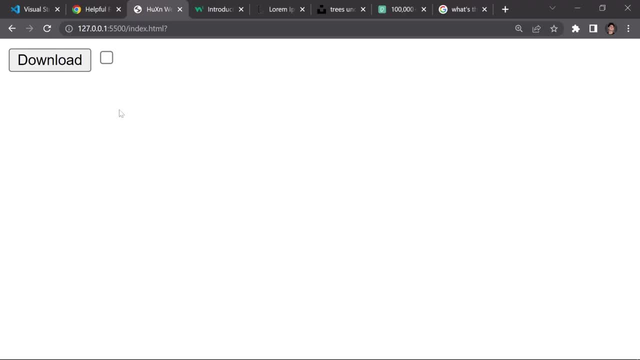 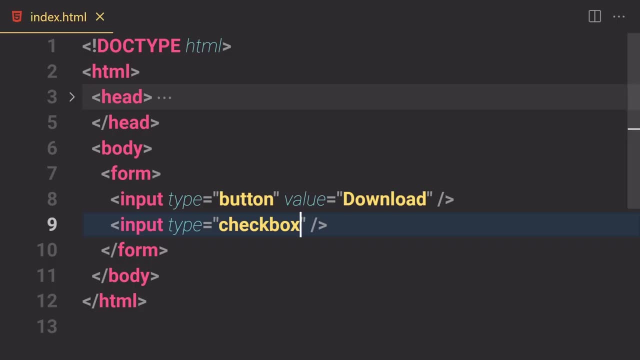 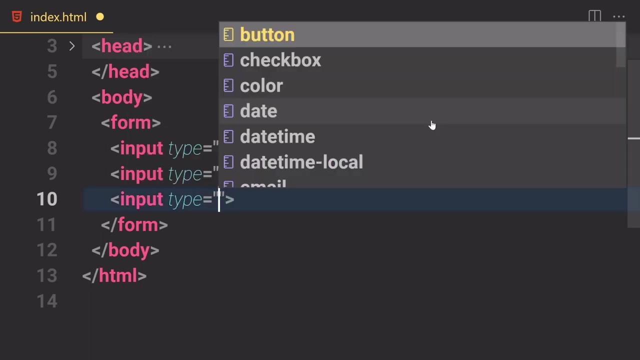 gives us a checkbox, as the name suggests. so save our file and boom, we get our checkbox right here. so if we can check it, we can also uncheck it and we can provide like more than that if you want to. so this is it about our input checkbox. now let's just create our new input of maybe we have like. 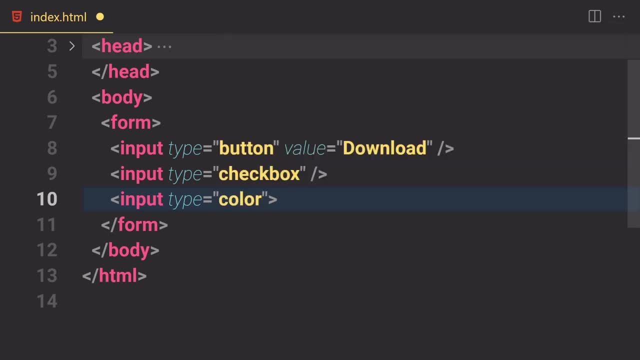 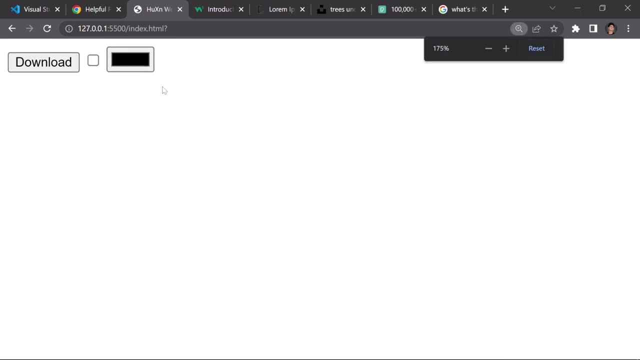 checkbox. so now let's just click on this color one- and this is my favorite one, to be honest. so if you save that and it will now gives us this color kind of picker right here. so here you can see- let me just zoom out a bit- so if you click on that, so it will not use us to change the color. 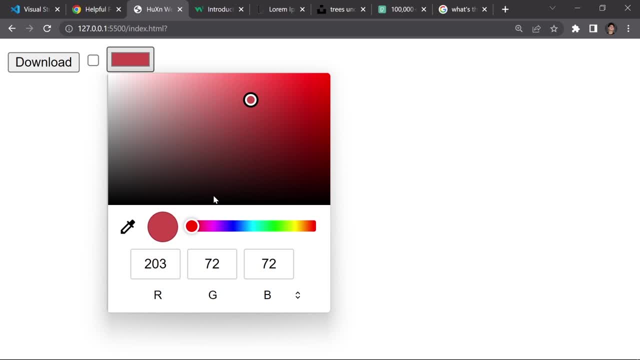 and we can provide our interactivity by using a javascript and it can give us a like crazy amount of color. we can also change this to from rgb to hsl, like hue, saturation, lightness, hexadecimal rgb and stuff like that. you don't have to worry about all of these colors and stuff for now. 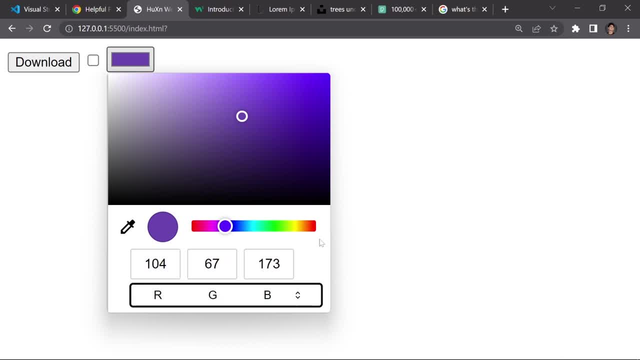 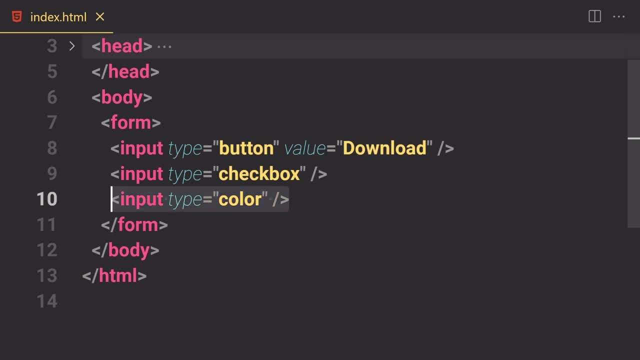 which we are going to be learning in a really, really, really great details. okay, so here you can see it. unlock uses a color picker right here. okay, so now, if you want to duplicate the same line so you don't have to select anything, you just have to hold alt, then shift and. 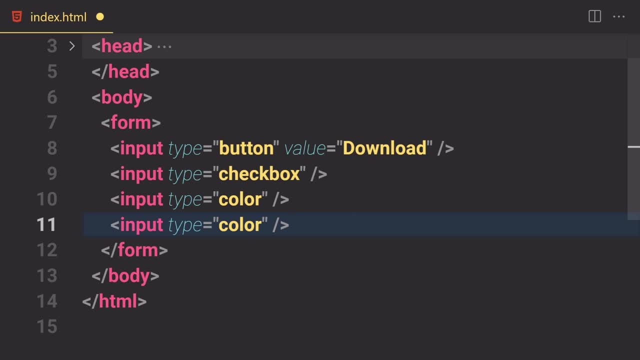 arrow. let me just say that one more time. if you want to duplicate a line like the line in which you're currently on, so you can use this kind of a shortcut in visual story coder- and i cannot guarantee for other kind of a quarter- you have to type it manually if it's not working on your. 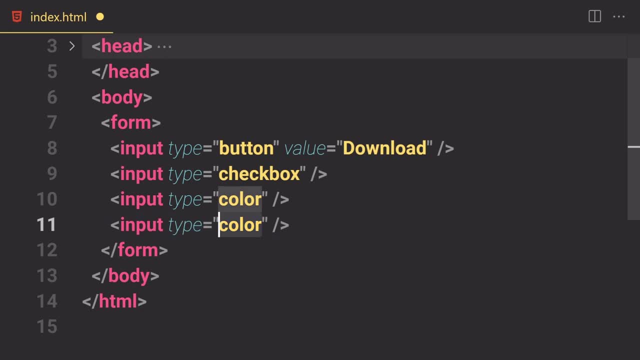 quarter. as i said in the beginning of the video, like if you are using a visual story coder, you're in a great phase. let me say that one more time: hold alt, then shift and then down arrow, so it'll just duplicate the current line which you're on if you want to remove the existing line. 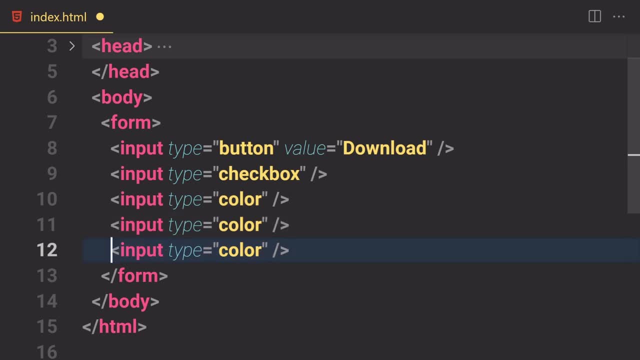 i know i'm giving your tutorial in visual story coder and i have entire course on that. if you want to check that out, so you know what, you just have to hold ctrl and hit exit. we'll just remove it from here. so now that was for a color one. now let's just select that and remove it. and now let's. 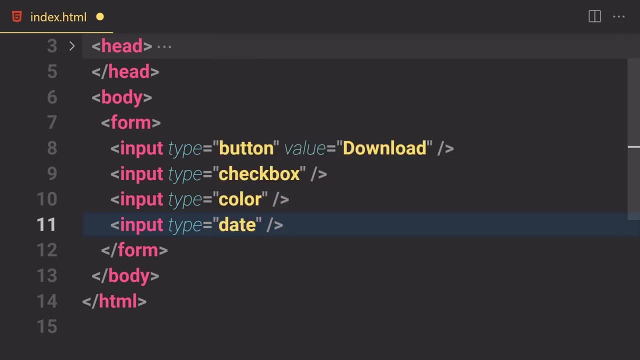 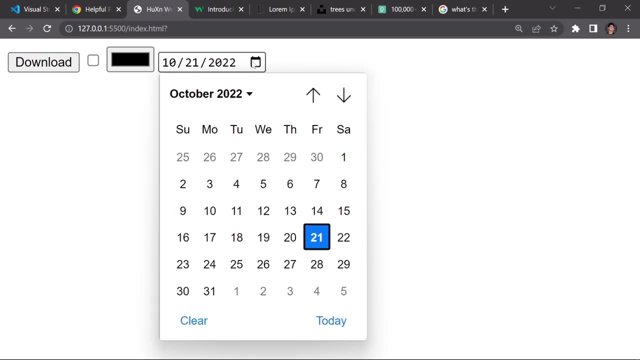 just select our date and, as them suggest, that it will allows us, it will not use these dead pickers, so we can just click on the today. it will not give us like 10, 21, 2022, and we can select a month and two, so this one allows us to provide a date picker right here, okay, so let me just duplicate this line. 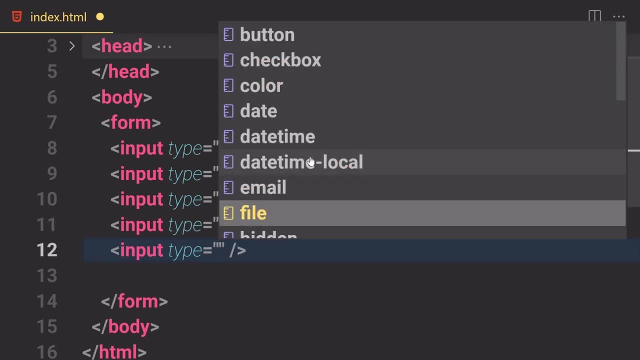 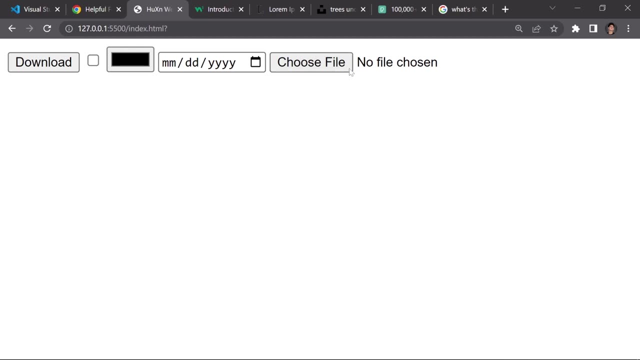 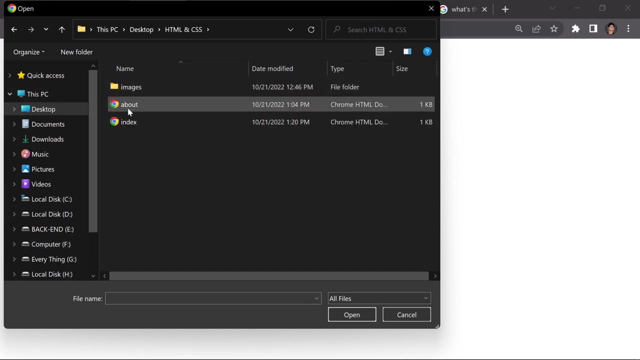 of code and here let's just select- or we already learned about email file- if you just click on the file one and if you select that, so here you can see, choose on file. no file has chosen, so if you just click on there, we can provide our file if we have one. so in my case i'm going to just click on. 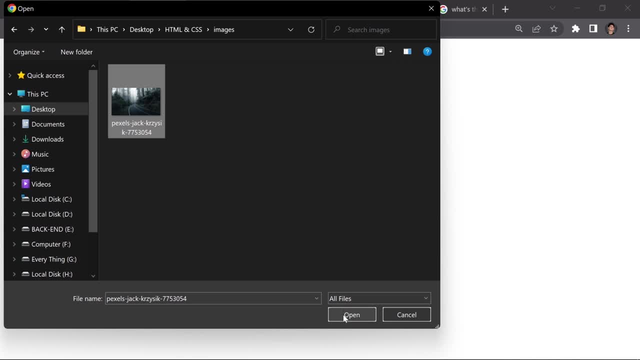 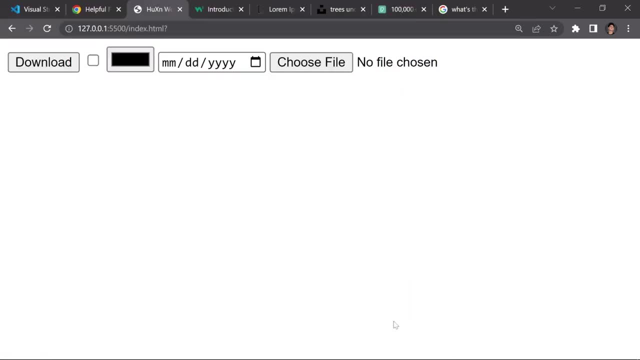 that and then go to the images and then we have that image which we downloaded just a second ago. open that and here you can see we have the name of that file. but if i click on that, click it one more time. that is gone because we didn't send our data to somewhere. 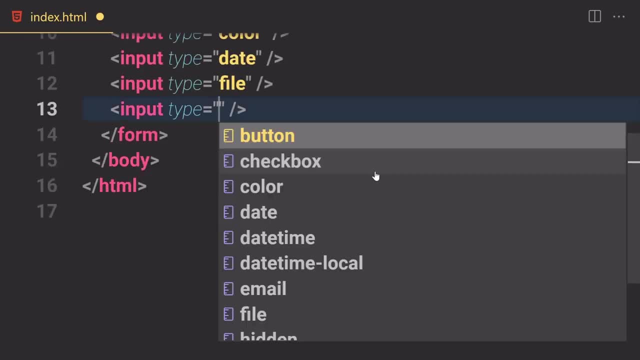 anyways. so now, if you duplicate that, and now let's just hit control space, and now let's just select a hidden one, it will do nothing. then we have an image, then we have a month. so as the time picker, as the date picker, we already saw that. so it will not give us a month, we can also have a. 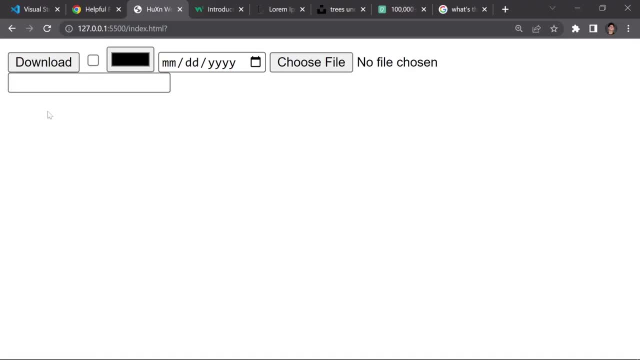 number one. this is a special one, so if you save that and now it will give us that same, put area right here. but here we are not allowed to write a letter just like a, b, c, d and gibberish like that. we can just only type an numbers, nothing else in there. so if i try to type something else, 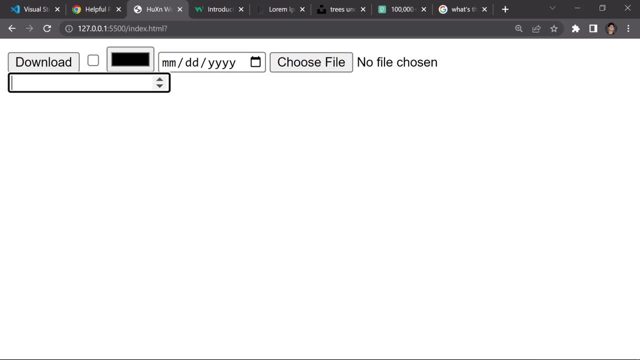 like you can also hear the noise of this keyboard here. you can see nothing is happening right now. okay, so that's because it is only available for numbers. so we can just put a numbers like maybe one, two, three, four, five, six, seven, eight, nine, blah, blah, blah, so we can just write a numbers in here. 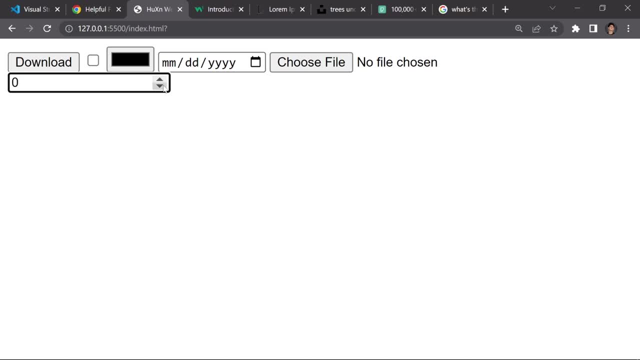 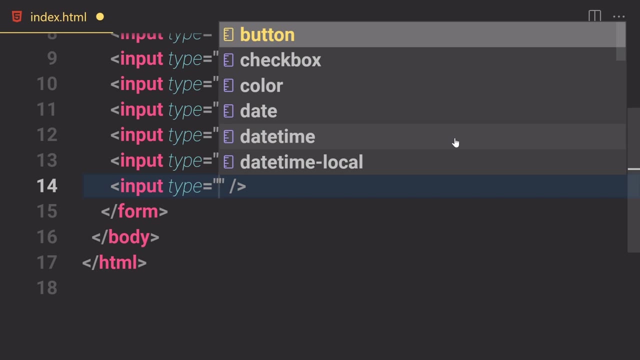 here and we can also increase or decrease. uh, and now let me just say the programming word. we can either increment a number and also decrement the number. okay, so we have minus one and stuff like that. so this is a number input. now let's just duplicate that one more time. and now let's just 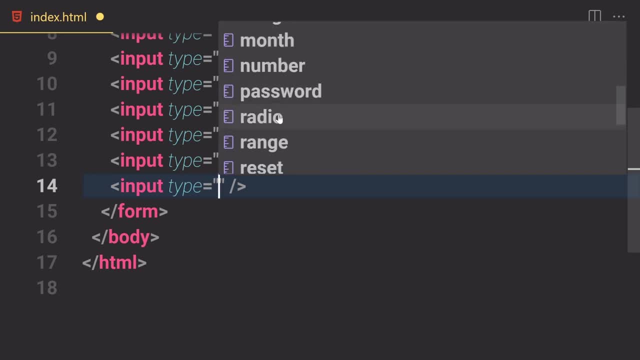 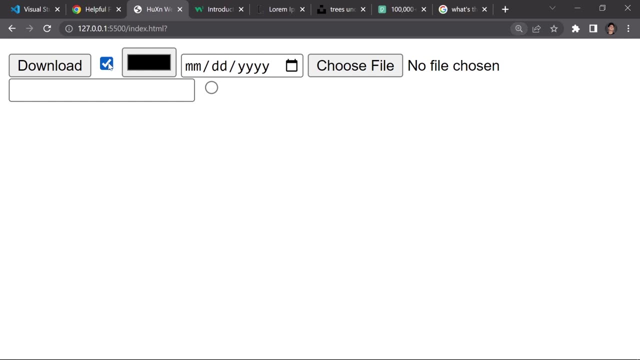 change that to maybe. okay, we got a radio buttons as well, so if you click on that and save it, and the difference between a checkbox and a radio buttons are, we can check and uncheck this box right here, but we cannot uncheck a radio button. once we check that, we have to create more radio. 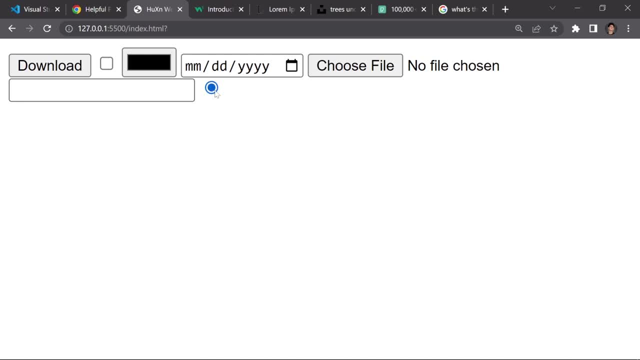 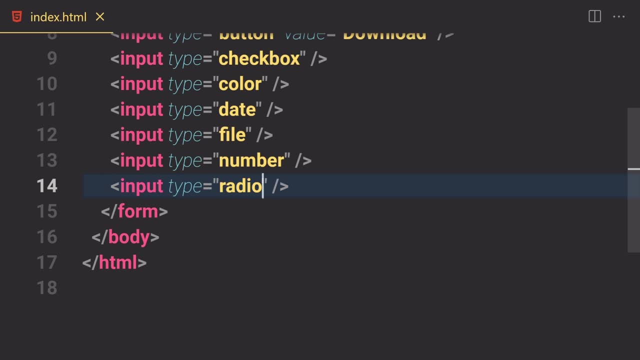 buttons to select the other one and we cannot like just remove that check box- i mean like the radio- from here, because we have to select something else. so this is how we can use a radio button. so now let's just duplicate that and select a range. so range is awesome. so if you save that, 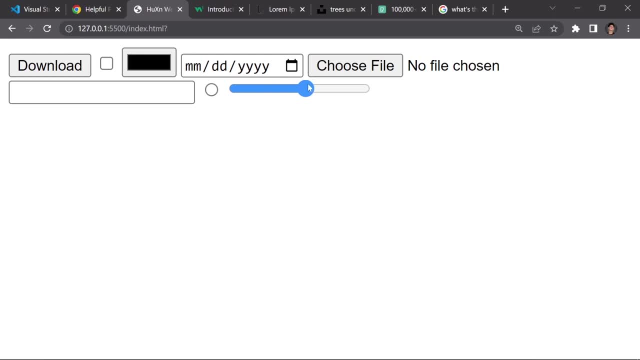 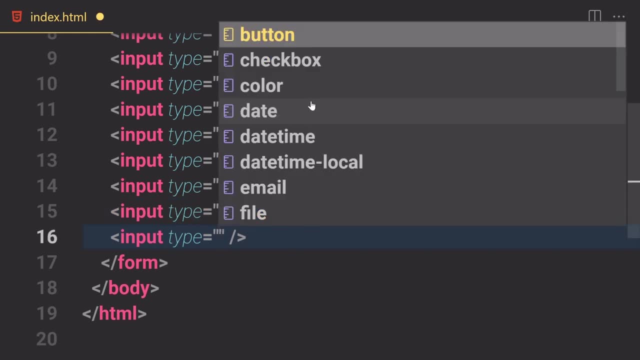 we can increase or decrease the volume or maybe the width and height of something. i have countless projects which is using these range. you can check out my project if you want to. so remove that, and then let's just select uh, reset, so, as the name suggests, there we'll. 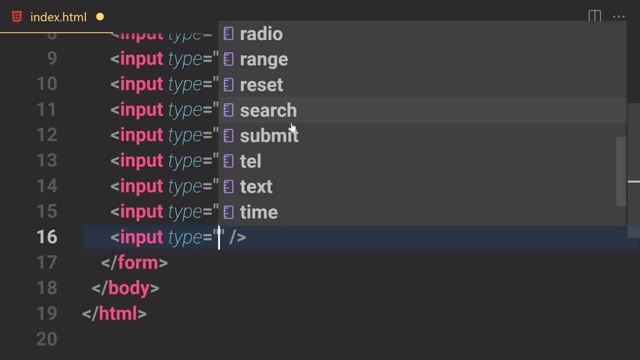 just reset all of the data which we currently have, and then we have a search, submit. we already learned about submit. we can also provide a phone number or tell- i don't know what's that even mean- we already learned about a text. we have a time which we learn url and then week, so we learn. 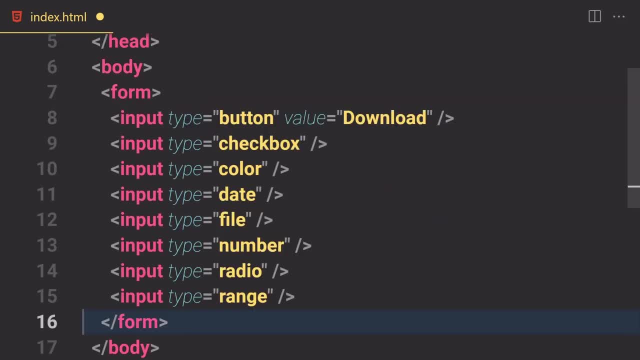 everything about that so you can just explore and play around with that if you want to in your spare time. but i don't want to waste my time, your time, so i just kind of want to give you like: where can you find all of that stuff? and it's on. 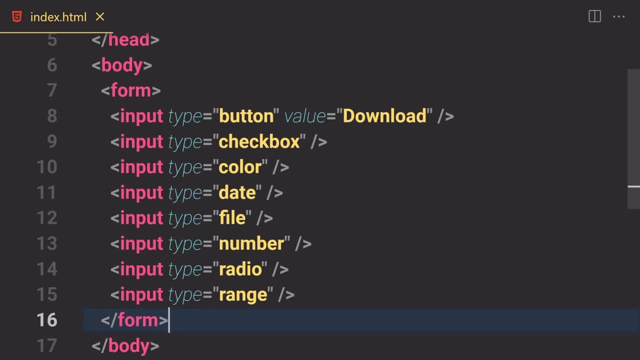 you to use it. okay. so now we are totally done with the forms in html. the next thing which we have to learn is what do we call it? a video and audio. so now that we know how to render image and how to render forms, so the next thing which we have to learn is something. 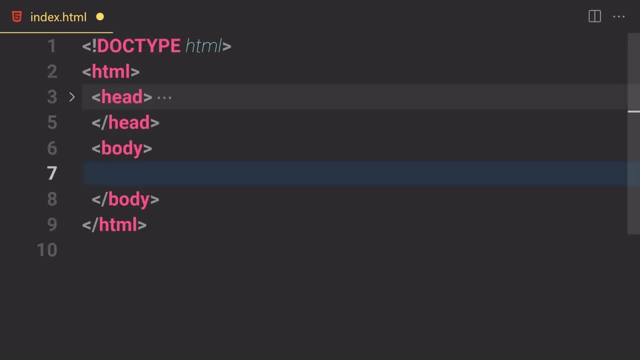 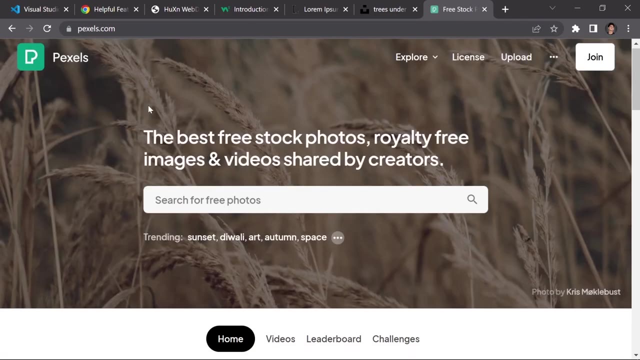 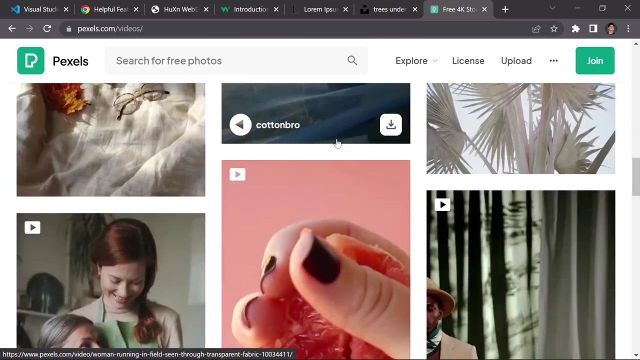 called radio and audio, so for that we would need to download some sort of a video or audio. so we are now in here, i'm gonna go back and here you can see we have these various right here so you can download videos from here, like high quality videos. but you have to give these people 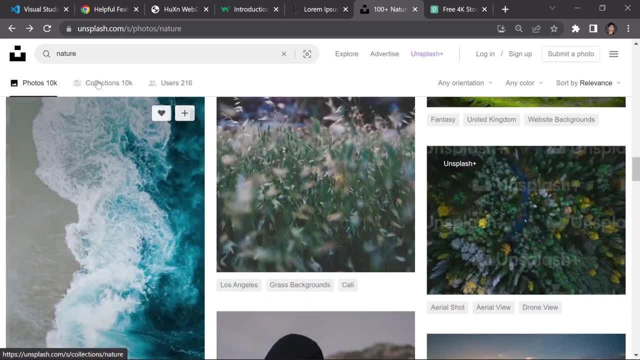 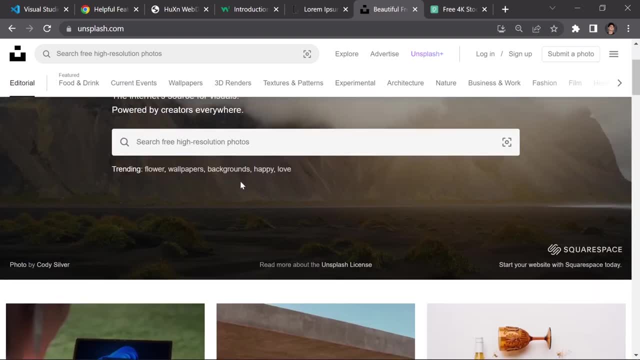 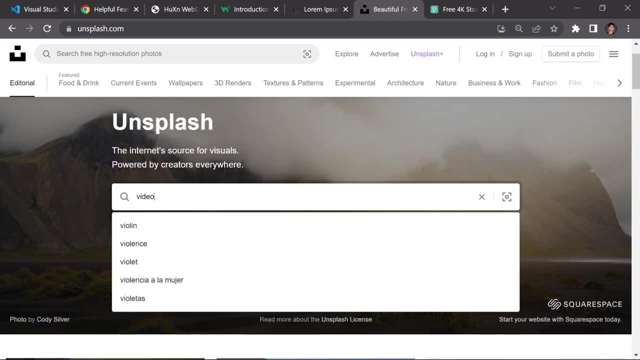 credit. okay, and you can also search, i guess, videos from this unsplash because they don't have any videos, i'm not sure, but i i guess they do have videos. okay, so happy love, blah, blah blah. they do have very, i saw that. so where do you use vrd e? 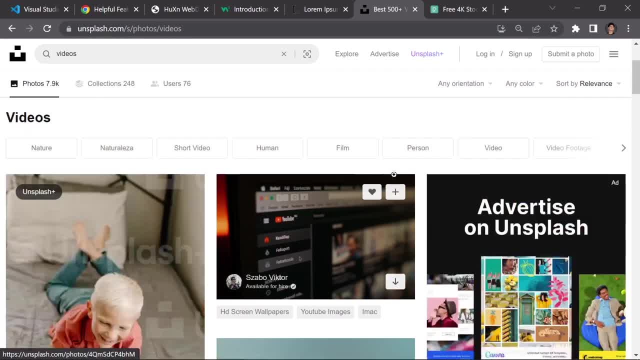 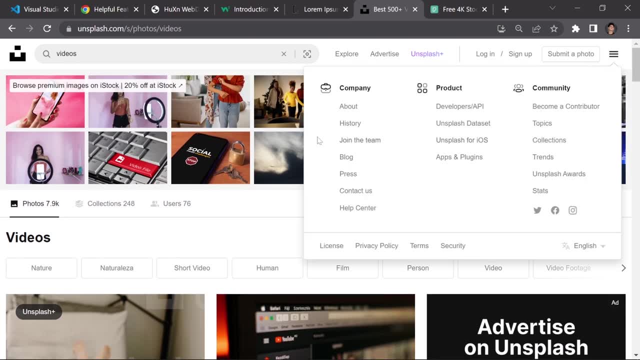 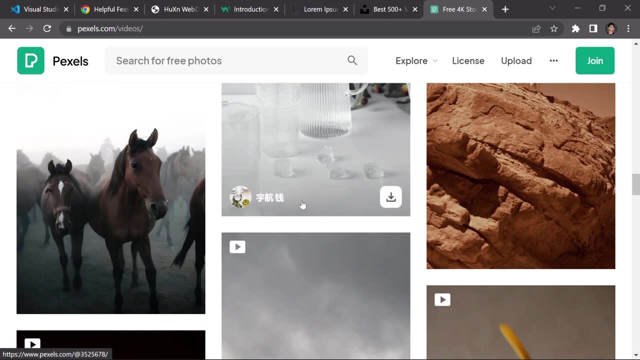 os. so let's just see. okay, i'm not sure if they have radios or not, let's just see in here, anyways, i'm not sure. so you are going to be downloaded. you can just download your radio from here, but just click on that. you can select a high quality radio and stuff like that. but 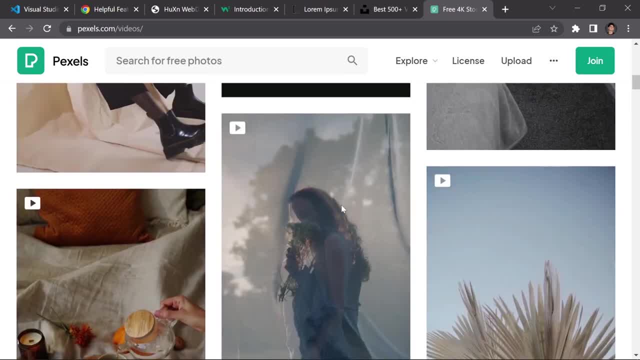 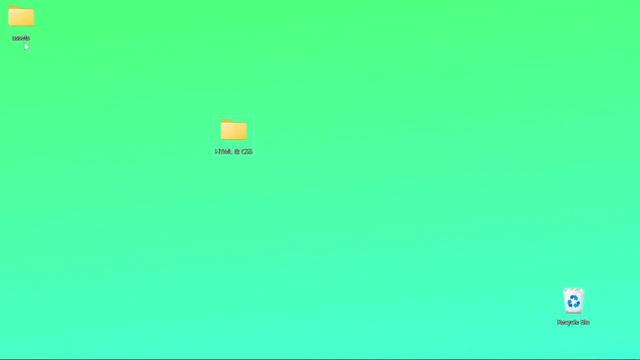 and so i'm going to just download a video in a second and then i'm going to come back in a second. so you just have to wait for me. i'm just kidding, i'm going to just flash through and then you will see that radio. all right, so i have now this assets folder right here. inside this assets folder i have 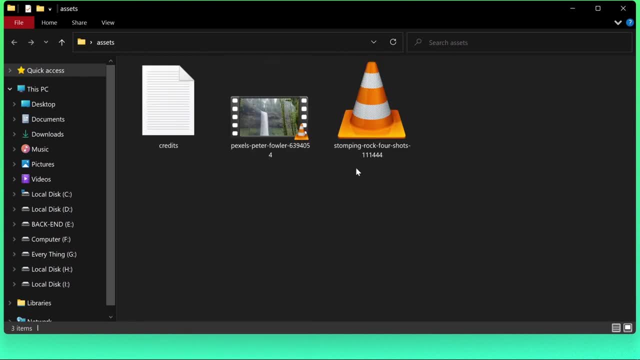 this, one radio and one audio. okay, because we are going to be using that. if you want to use the same audio and radio which i'm using, so you should have to just click on the link which i'm going to provide in the description below and you should download that in my github repository. 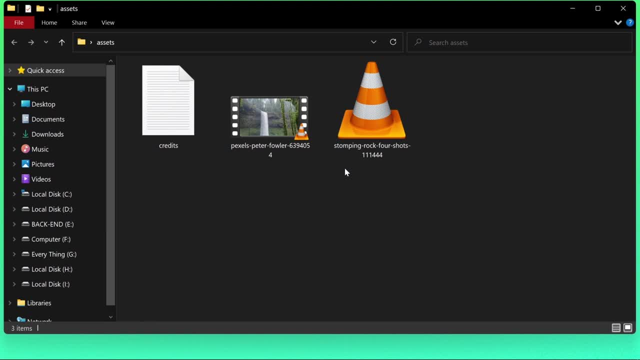 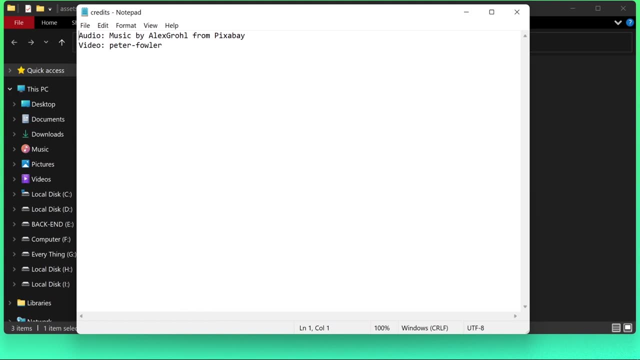 if you don't want to use that and if you want to use your own images. so you are totally free to use whichever kind of radio or audio you like. it doesn't matter. and here let me just show you the credits. so credit for the radio goes to this kind of a guy. sorry, i can't pronounce your name. 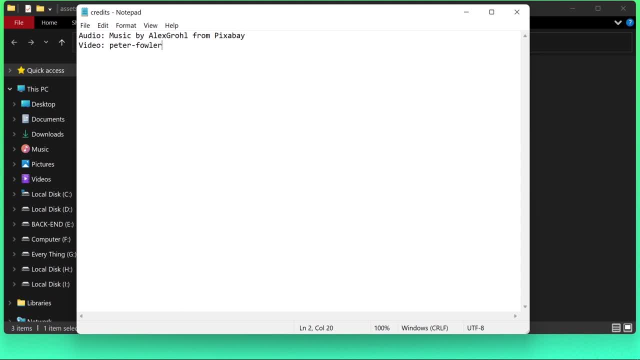 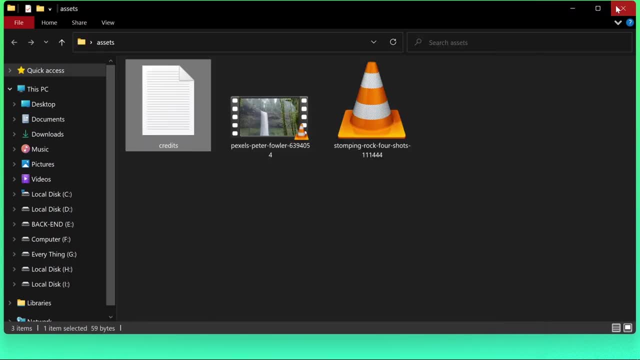 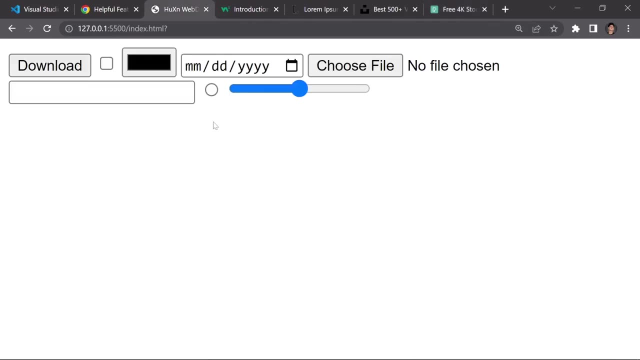 and this where you came from this pixie b, and i guess this audio came from somewhere, but i'm not sure anyway. so we have this assets folder. so what do we have to do? i'm going to drag this folder into my html css directory right here. so let's just hit ctrl b and we have this assets folder. 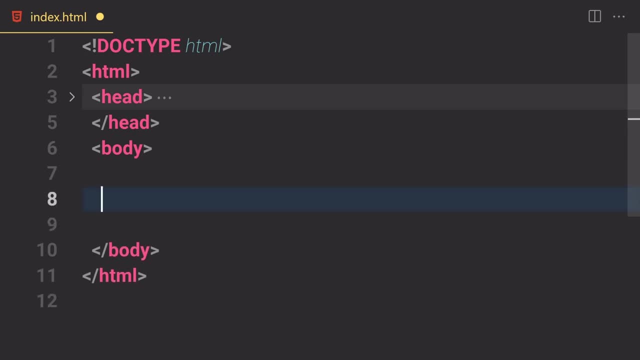 right here. okay, so now, if you want to render audio or radio, so for that you just have to first of all write a video, and if you hit tab it will ask us for a source of that video. so what do we have to do? we have to just hit ctrl. i mean like hold ctrl and then hit space. and here we have to select. 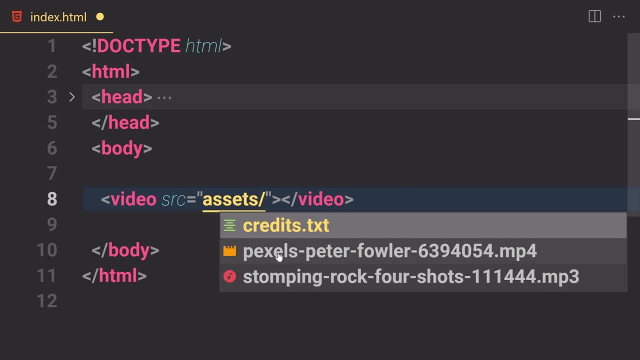 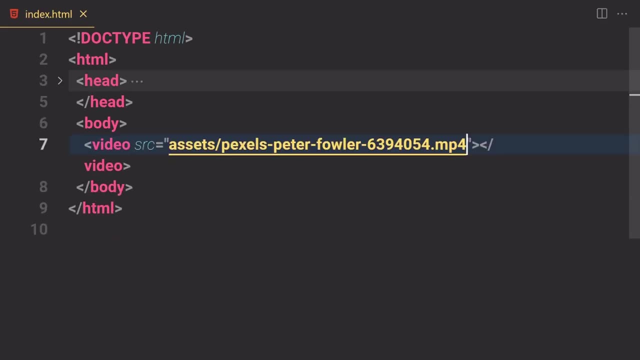 our assets folder and then, in this case, we are interested in this radio, so we can just click on this radio, okay? so let me just zoom out a bit so you guys can see everything a bit better. and now if you save that, and now if you check it out, 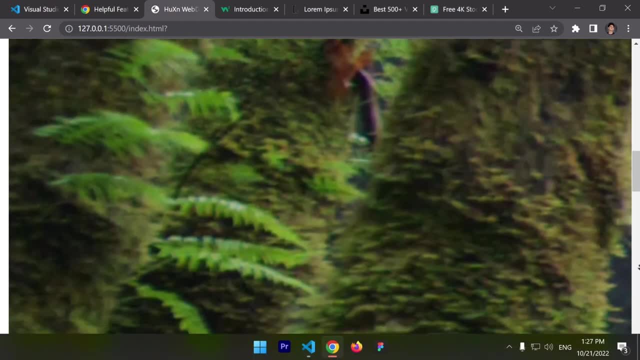 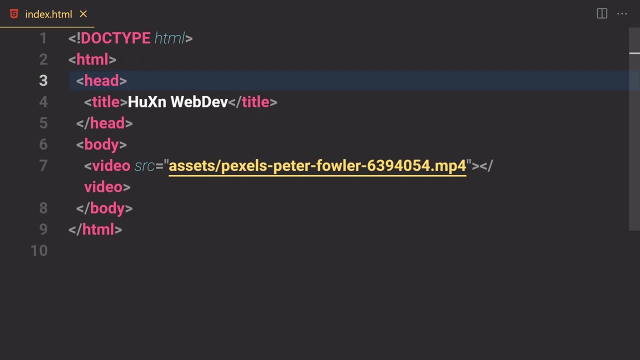 so we are just getting this image and this is also massive. so we are going to be writing internal css and you don't have to worry about anything which i'm writing inside or underneath this title right here. okay, you don't have to worry about anything right now. so, basically, what we are doing. 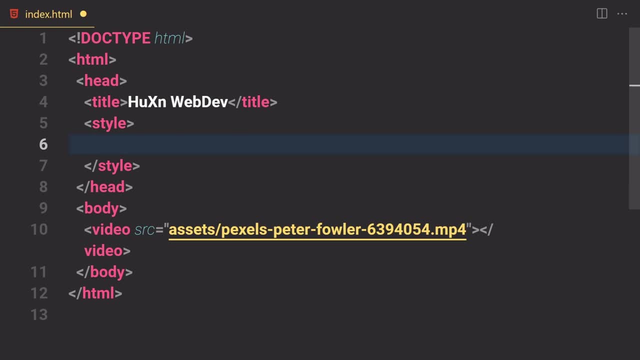 is that we are just shrunking down the size of that image. so first of all, let me just get my radio and let's just write a width of maybe like a little bit of a width of: maybe like a little bit of a width of, maybe like a little bit of a. 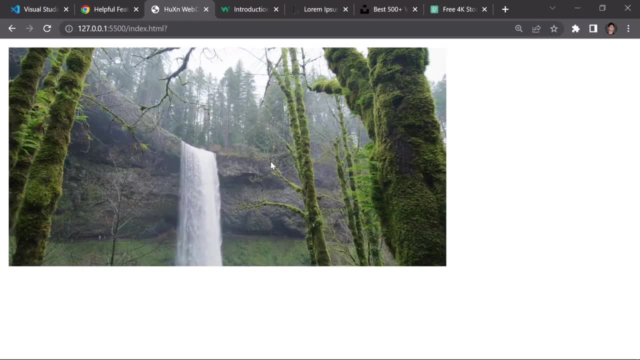 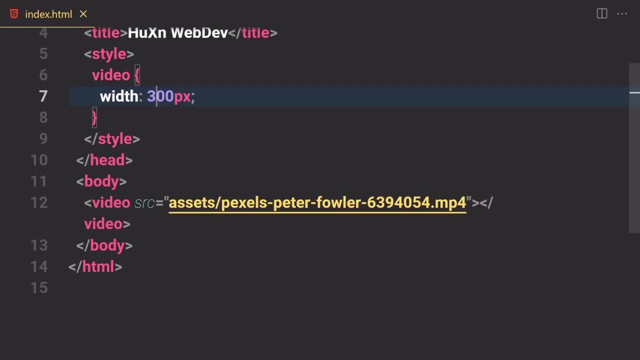 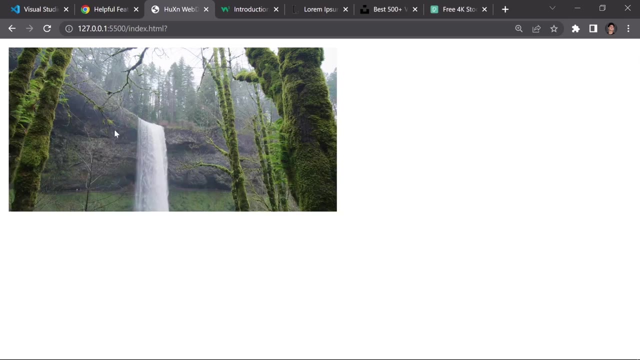 i don't know. 400 pixel define server, and this is how it looks like for now. oh, you know what 300 pixel would do? yep, that's cool. okay, so now. so this is known as internal css, which you don't have to worry about it for now, because we are currently learning about html. and now here you. 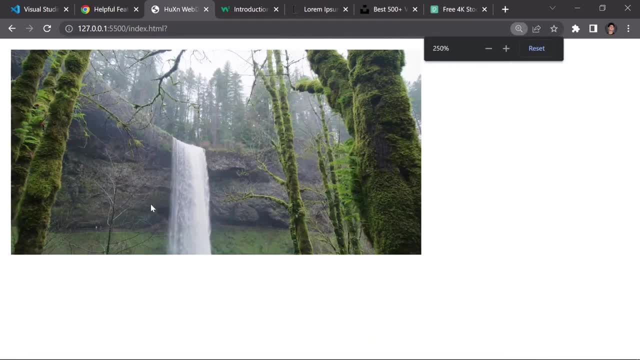 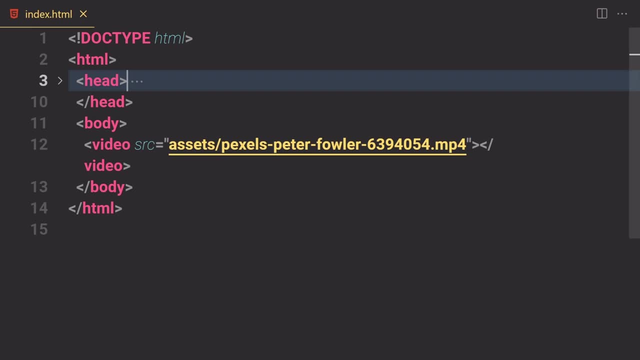 can see. this is just an image. it's not a video like. we cannot play it, we cannot pause it, we cannot increase the volume and stuff like that. so if you want that kind of controls for this video, so what do we have to do? just type in the name of the video and then we are going to be writing. 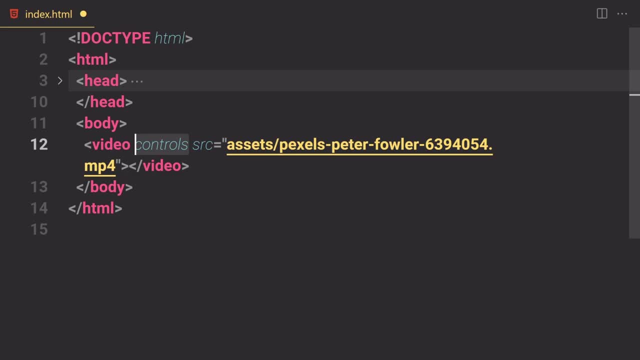 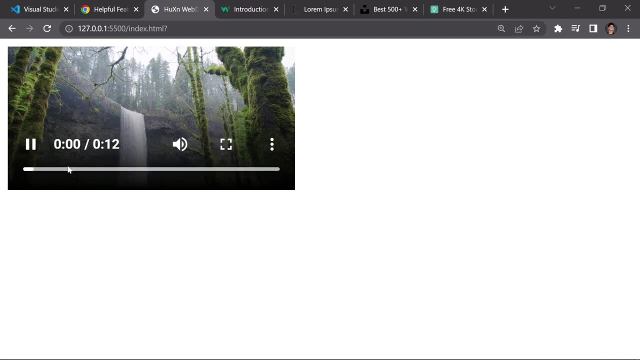 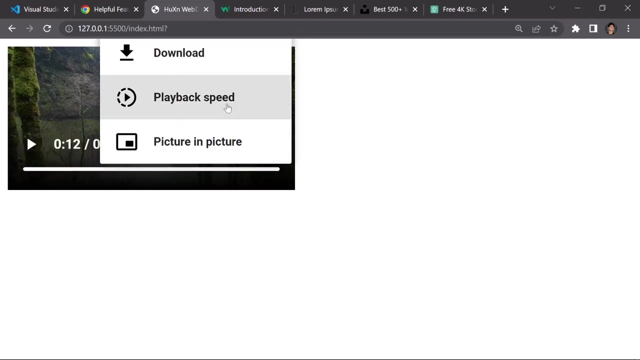 a controls attribute right here. okay, so if you save that and boom, we are now getting all of these kind of stuff like. we can full screen it. we can play the video. we can increase or decrease the volume if you want to. we can full screen there. we can also download this radio into our machines. we. 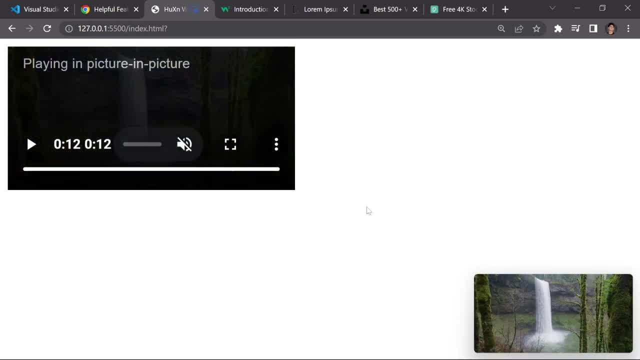 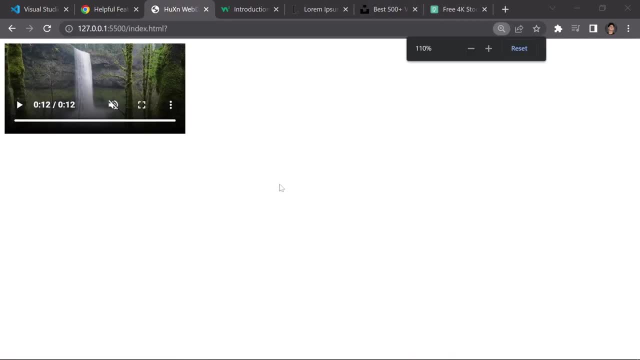 can also go picture to picture. so if you just go to picture to picture, so like we can visit the other side and we can also see this where you're playing in here and crazy stuff like that, so here you can see the log users and you can see that we have a lot of different things that we can do. 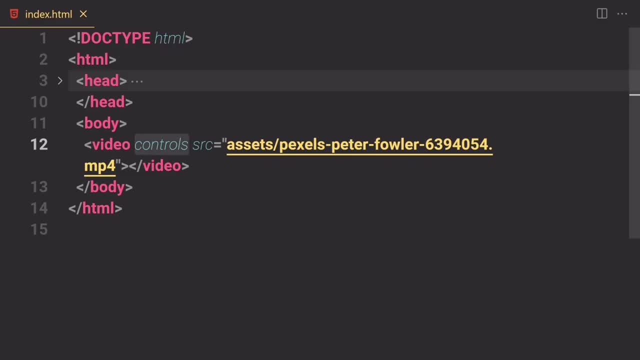 controls right here. okay, so this is because of these controls attribute. now this is about a video: how to render a video. now let's just learn about how we can render audio. so it's kind of a symbol, just like a video. when you start writing a video, you just have to write like a audio, right? 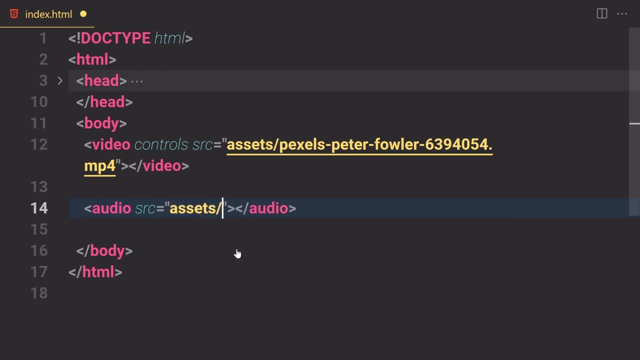 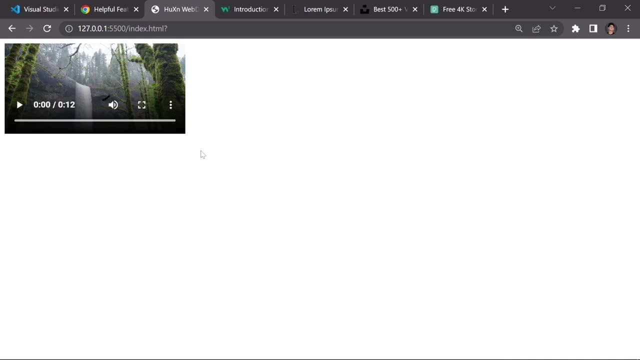 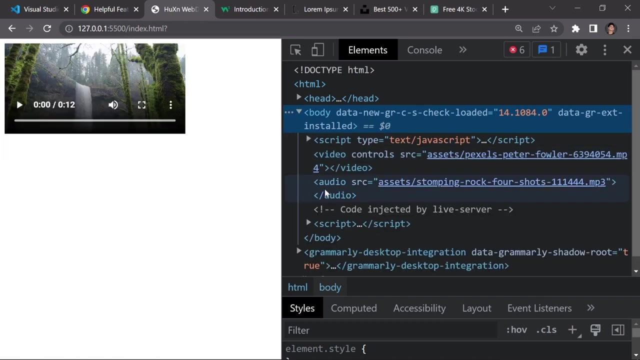 here and specify the source, hit control space, then go to the assets folder, then click on this kind of uh, storm rock, whatever. so if you save that, we are getting nothing. why, if you just right click on it and go to the inspect area right here, we do have that audio right here, but it's not showing anything. 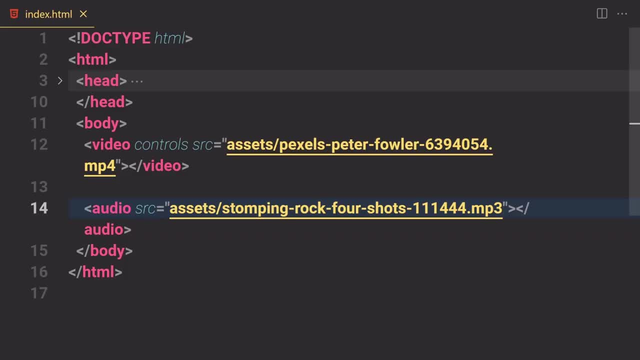 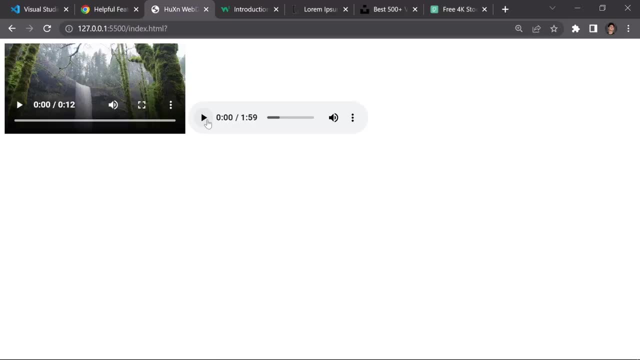 that's because we don't have controls for that. and if you want that control, so we just have to specify it right here. so controls, and if you save that, and now here you can see, we are now getting these controls, so we can play that. it's kind of a crazy voice, so we can just 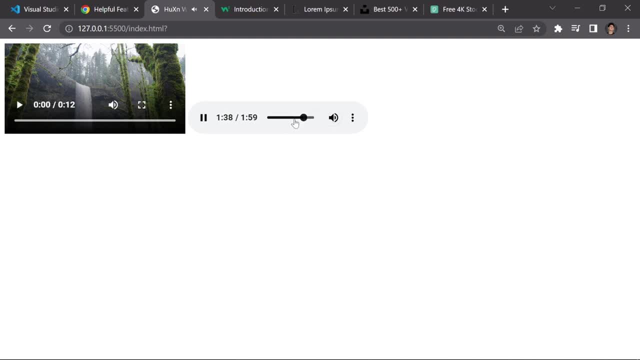 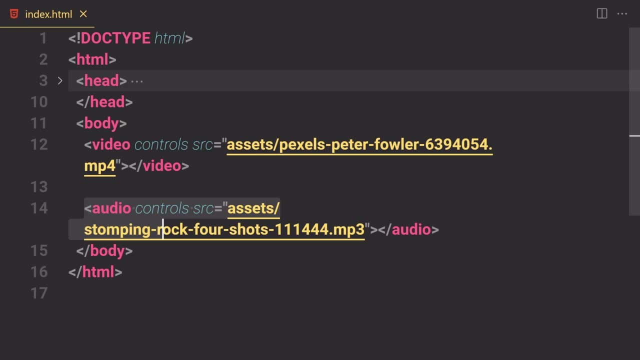 uh, make it a bit slow, we can play it one more time, and stuff like that. so this is how we can render video, this is how we can render the audio, and we already learned about how we can render images by using html, so i'm going to just remove all of that from here and now the next topic, which 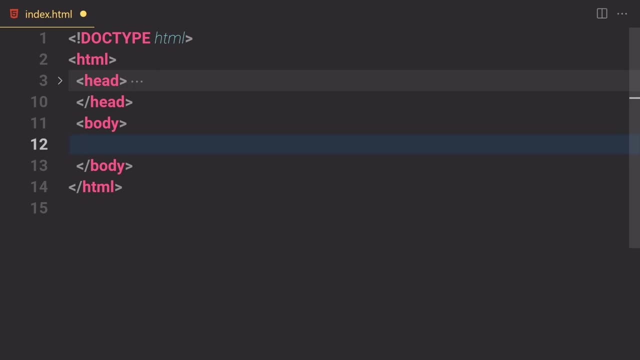 you are going to be learning in this video is something called a semantic html. it will not show us the results, but we have some other language, so now you might be thinking like we already learned about html which stand for like hyper text, markup language. so what is that semantic html even mean? 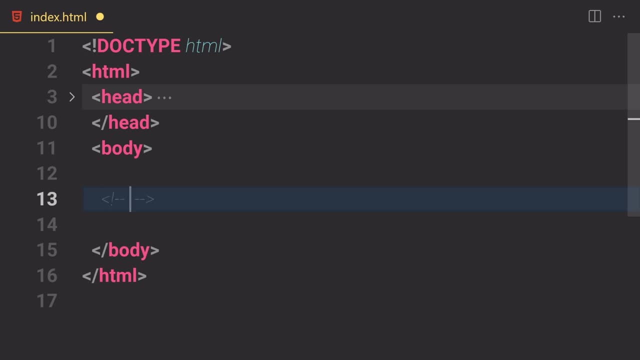 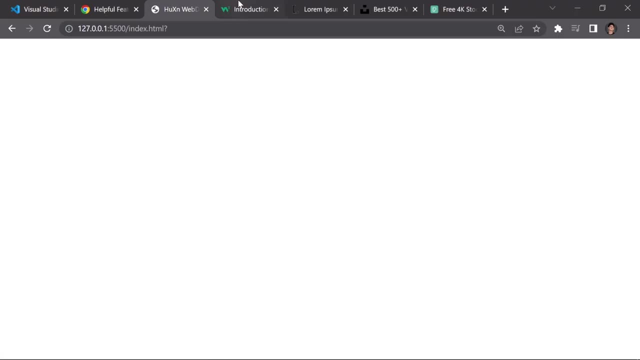 a semantic html. semantic just simply means meaning so if you just write like: uh, you know what, let me just show you the you know docs, then you'll get to know what i'm talking about, and i'm going to remove that from here. lorem ipsum as well, go back. 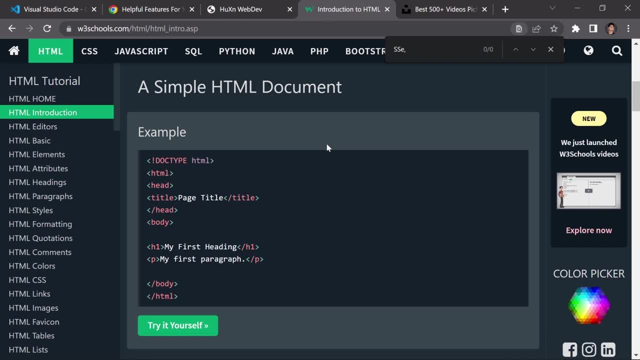 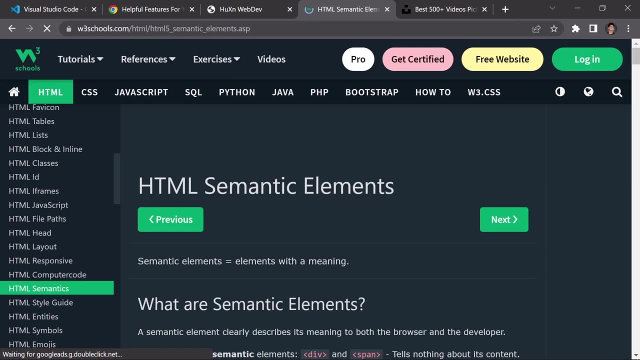 and here, what do we have to do? i'm going to just write s e m and okay, s e m a n, and here you can see we have a semantic html right here. if you click on there, you have. semantic html is nothing but just a new tags right here, okay, so we are going to. 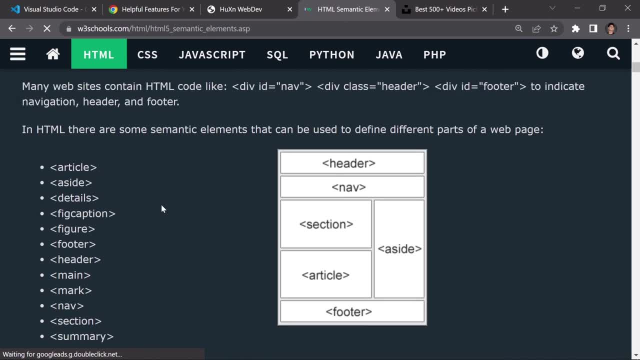 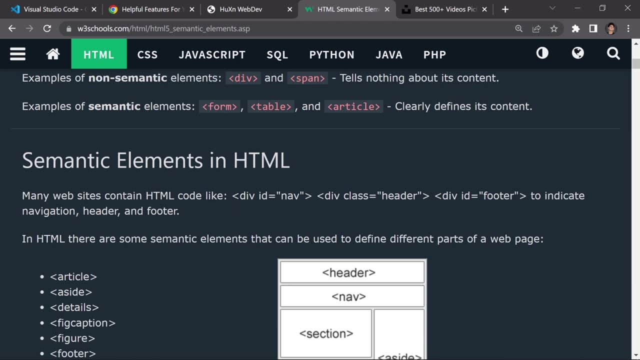 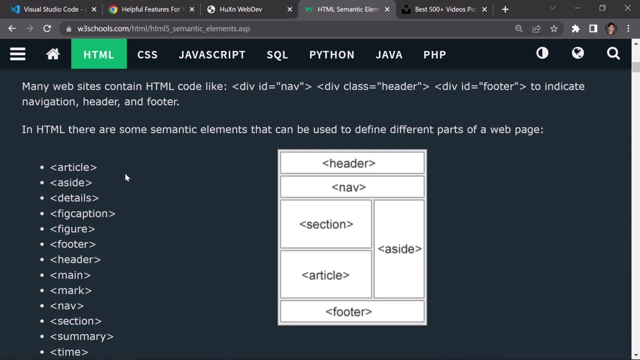 be learning about these new tags, which allows us to like better structure or html documents. so what are semantic elements in html? many website contains html code like um, div and then id. you don't have to worry about that. david the classes and in indicator, navigated header and footer and stuff like that. in html there are some. 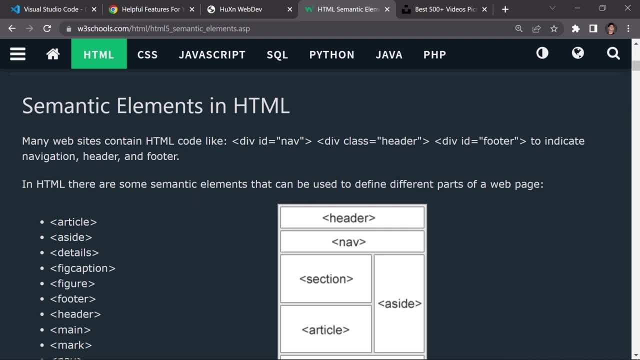 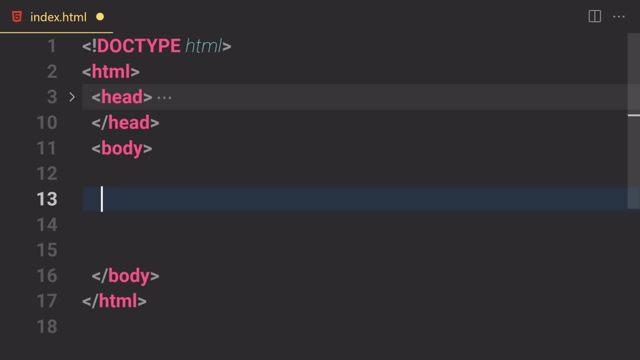 semantic elements that can be used to define the different parts of your web pages. so, instead of a div and span- and now let me just show your div and spans- and we are going to be using a lot of div and spans, div and spans, and this is not a better way to structure your code, like we are. 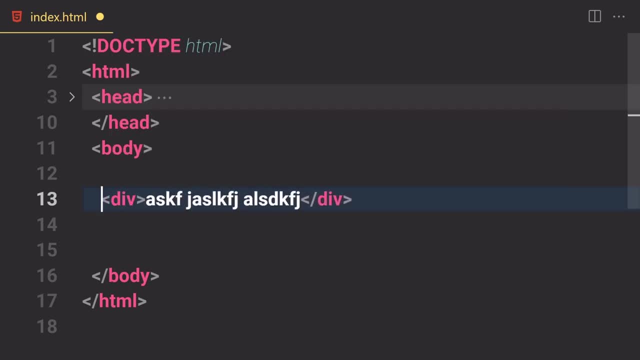 going to be writing a div and we can type anything inside there and it's just a container. it's just a container for writing your code or just putting your content. and then we have a span and we can also write anything inside there. both of them don't have any meanings to it, but both of them. 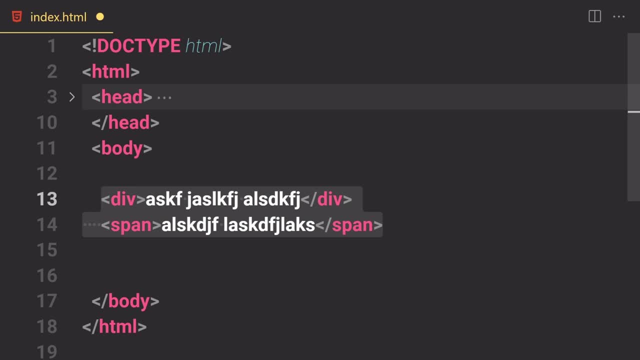 are the most useful ones in html document. so we don't have- we as a programmer don't have- a lot of time to just write like section or just write like article, because we are supremely lazy and that's a bad practice. so we just write like div and we also write a spans, and that's because of. 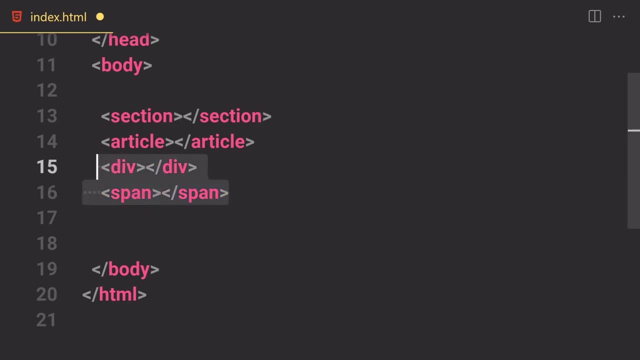 time consuming, and this is like these two are like a bad way to write our code. i shouldn't have to say bad, but we are going to be using that a lot, but, um, it's not a better way to structure your code. if you want to structure your code so you can use a. 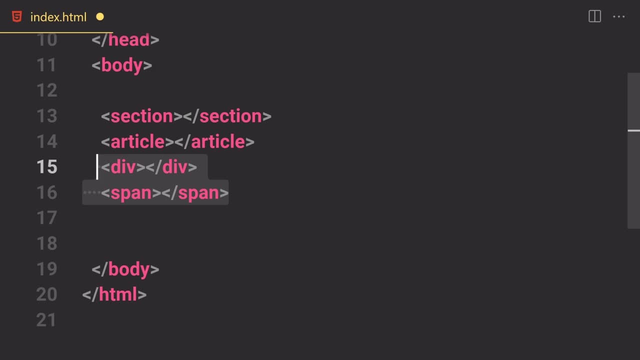 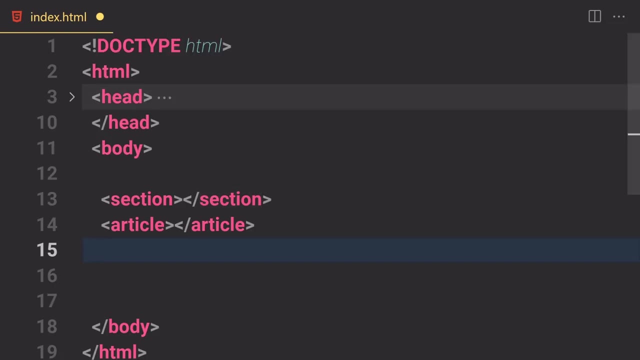 semantic text. both of them will work like div and span will work, but it's not like a better practice for other developers to write your code like that. okay, so in maybe like one years later or maybe some time later, like other developer come into your project and they see, like all of the div. 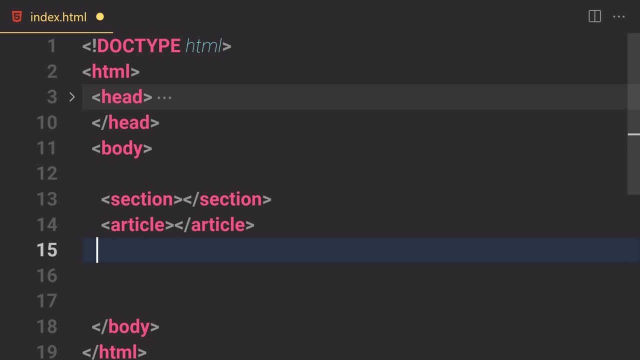 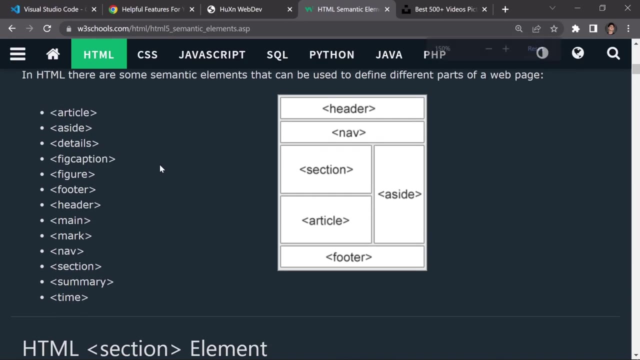 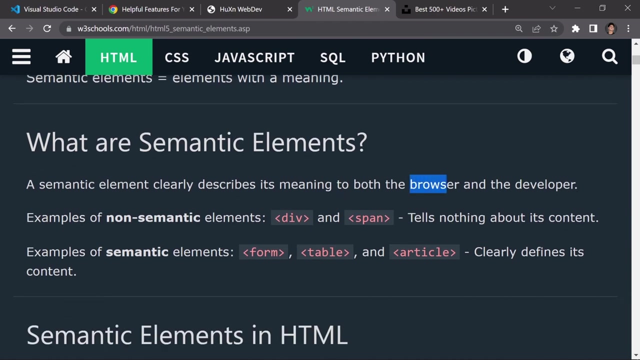 span, div, span, div, div, div, div, div. so they'll be like: what the hell am i looking at? okay, so for those programmers, you just have to write like section article and stuff like that. you have to use something called a semantic element. so a semantic element clearly describes its meaning to both the browser and also to the developer. okay, so by browser we 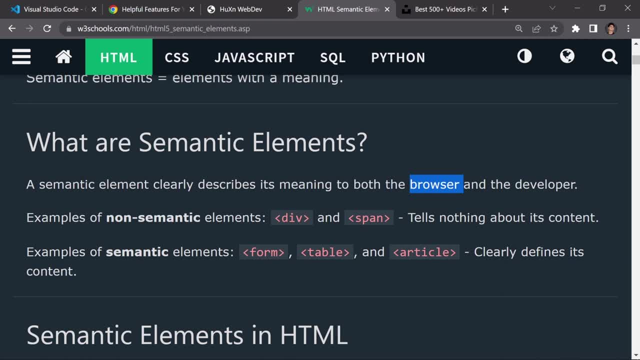 means like seo, performance and stuff like, in which i'm not going to go into that much details, but uh, it will just describe its meaning to the browser and to the developer as well. example of non-semantics elements are like, as i said, div and spans, and we have, i guess we don't. 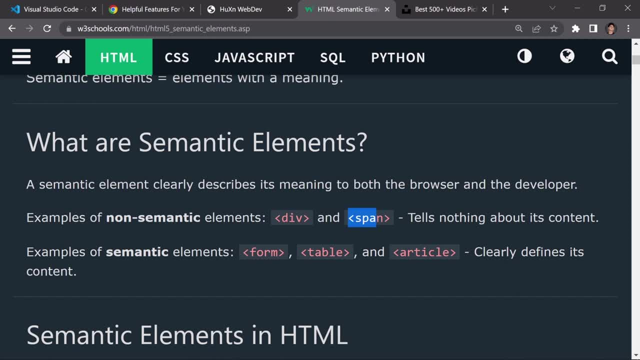 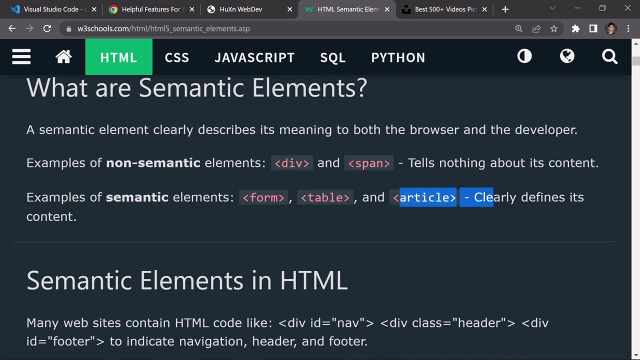 have any other non-semantic elements and tells nothing about its content. like this. stuff like div and span doesn't tell about nothing. that doesn't tell nothing about its content. so example of semantic elements are forms as we learn, tables we don't have to learn, and then article and stuff like that. so here are just a few. 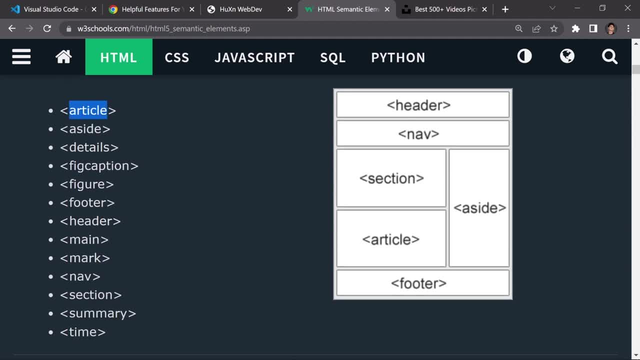 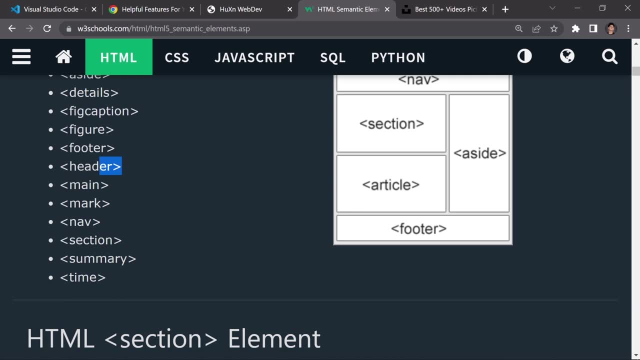 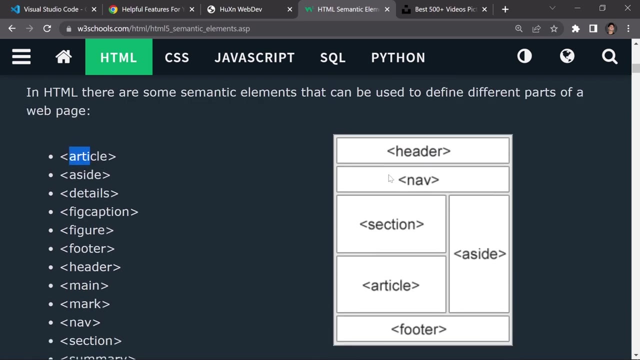 examples like of a semantic element. so we have article, we have a side detail, the caption, figure, footer, header, main mark, uh, navigation, like a nav section summary, and so before getting into the details of any of them, first of all let me just write like: okay, so we 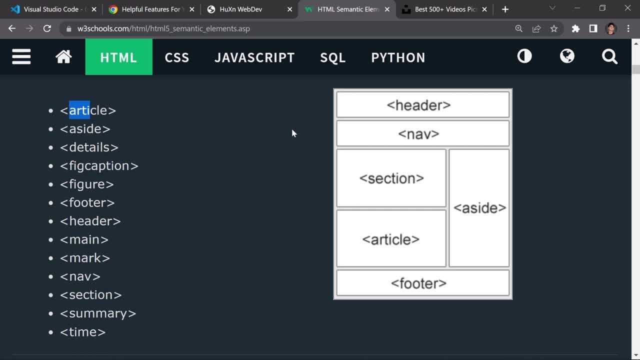 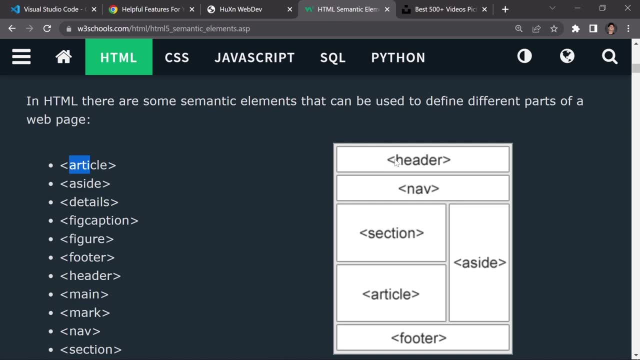 already have this example. so if you want to structure your website like first of all you would have a header or a hero area, so for that kind of thing, instead of writing a div we can just write a header area, or just write a header opening tag and header closing tag and then 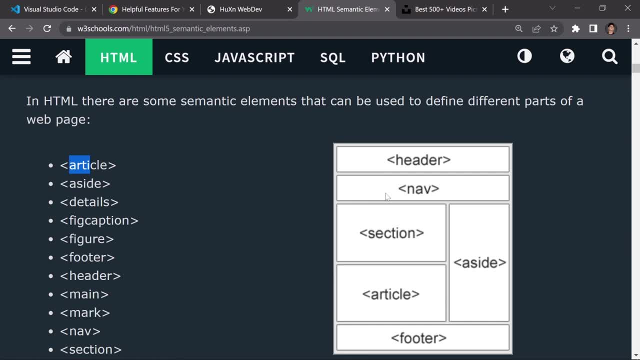 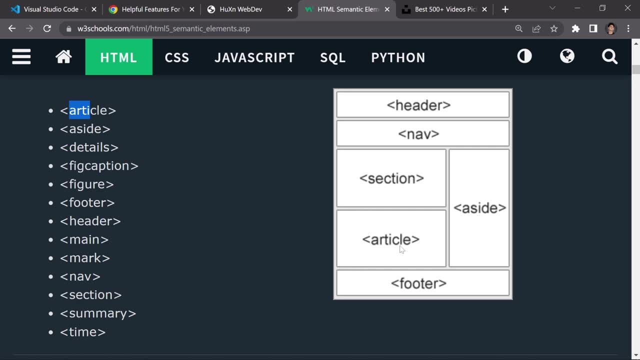 instead of writing a div or span, and so for navigation we can just use nav and we can also have section inside a section inside a section. then we have article, we have a side and footer and all of this kind of a crazy terminology which you don't have to go into that much in detail. 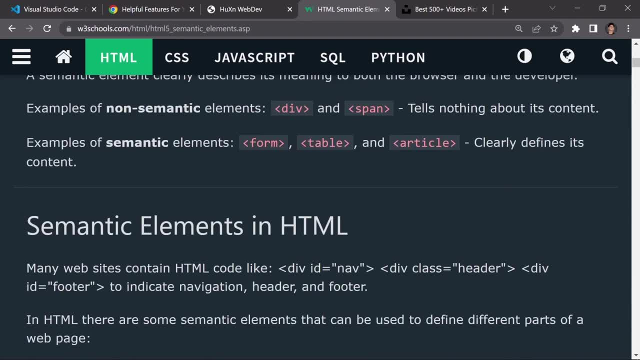 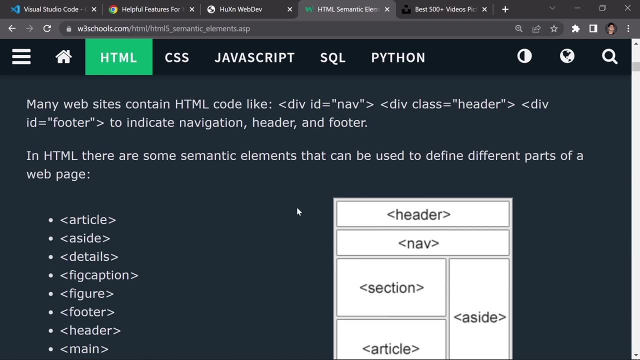 but you just have to remember that a semantic means meaning, like we are going to be writing a meaningful elements. so now let me just give you a quick example of that. first of all, you know what? what should i do? uh, okay, you know what. i'm going to just ask from google instead of showing you. 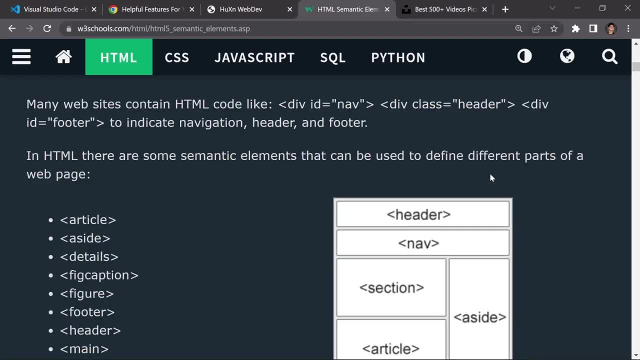 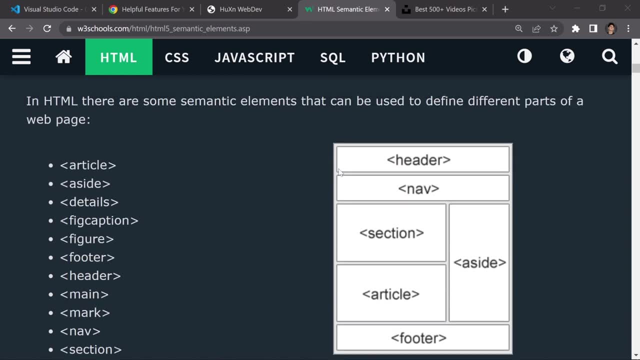 the figma files. uh, oh, you know what? i'm going to show you the figma. i'm going to launch a figma right here so i can give you a better example of that and you can use the semantic elements for yourself. but it will take a little bit of time to render. 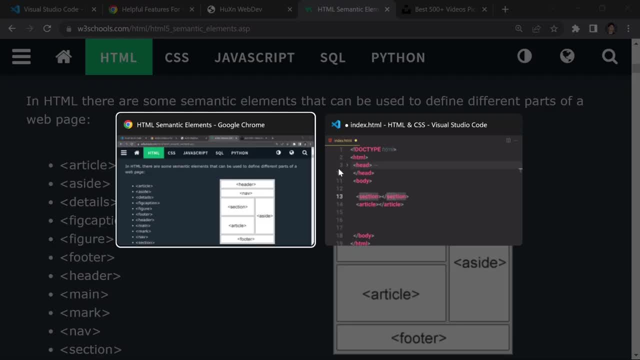 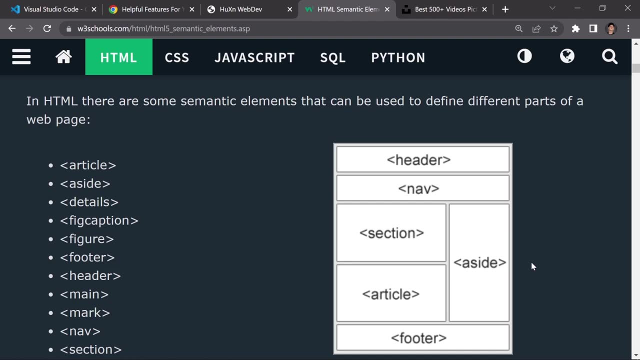 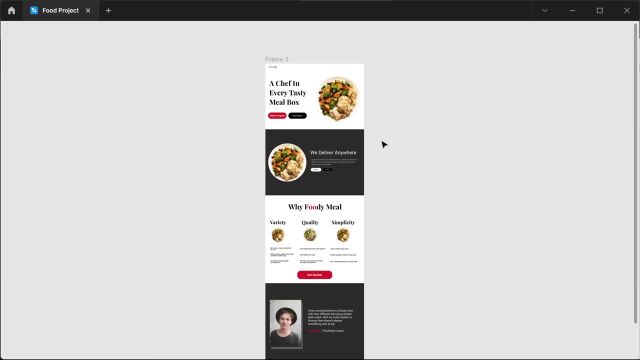 but it will take a little bit of time to open a figma because it's nowadays a little bit huge to open my and my internet speed is very low in this area. i'm gonna have to switch back over to some other area, but for now we have to wait for a figma to render. suppose we have this uh website. 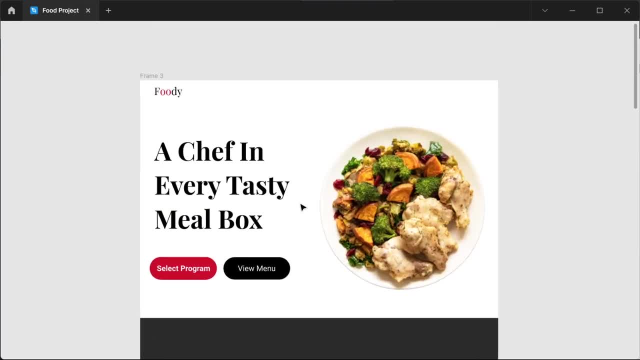 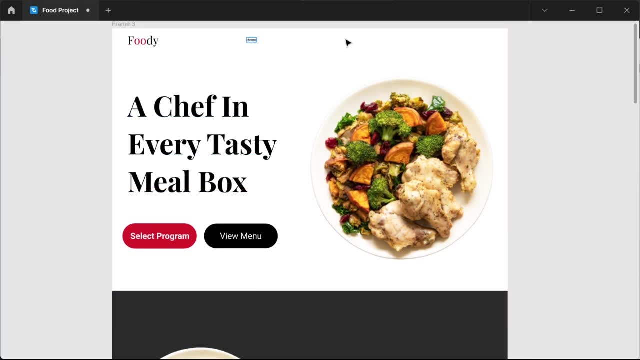 right here and we're going to write a figma, and we're going to write a figma and then we're going here and we're going to be maybe building this website. so, first of all, what do we call this area? we can also have or on home, and we can also have or a section. you don't have to worry about this. 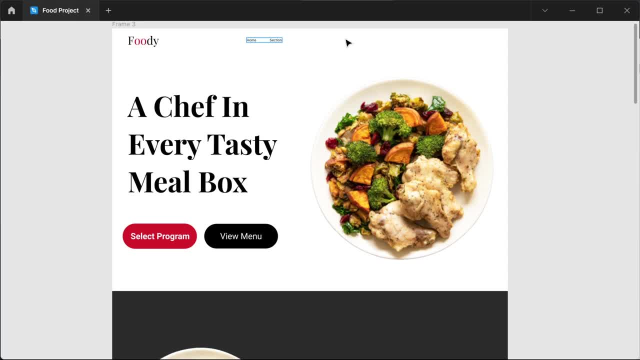 software for now, because we're not going to be using this software in your course, but i just kind of want to give you just for demonstration purposes. so we have section and then we have about section and we have maybe project section or stuff like that. i'm going to just make that a bit bigger. 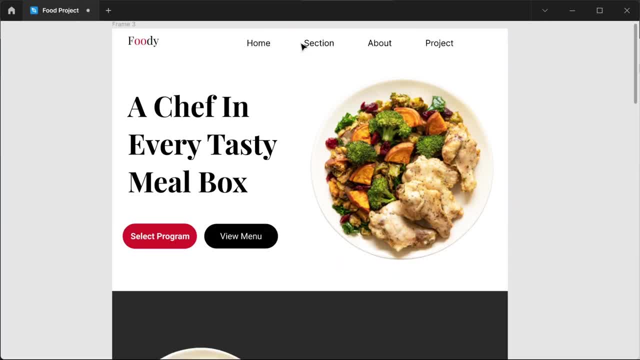 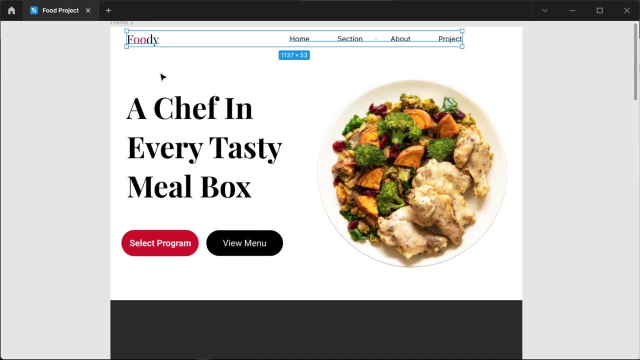 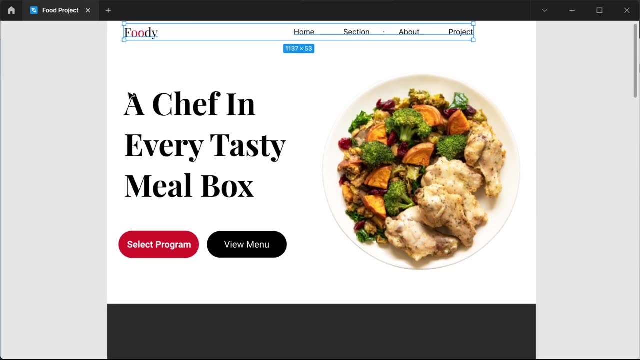 okay, let's just close that one and i'm going to make it bigger so you guys can see everything a bit clear. so here you can see. first of all, this area will be, or navigation for our project. okay, so let's suppose we are building this website, so this will be the navigation for our website, and then this area will be known as a. 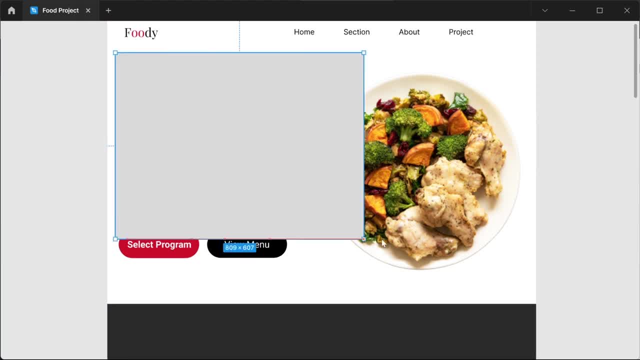 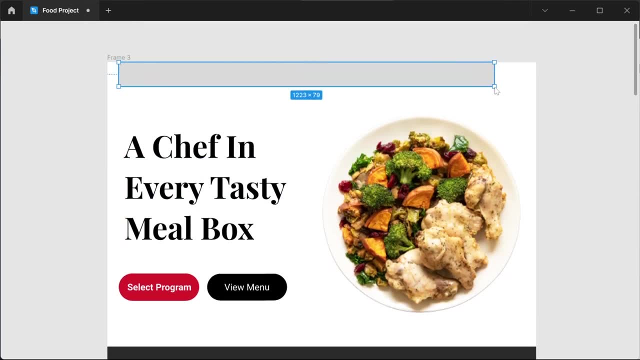 header area, or you can also call it a hero area. let me just write it: this area will be our hero area and let me just move there real quick, and this area will be our navigation. so i'm going to just give a name real quick. i'm going to just give a name real quick. i'm going to just give a. 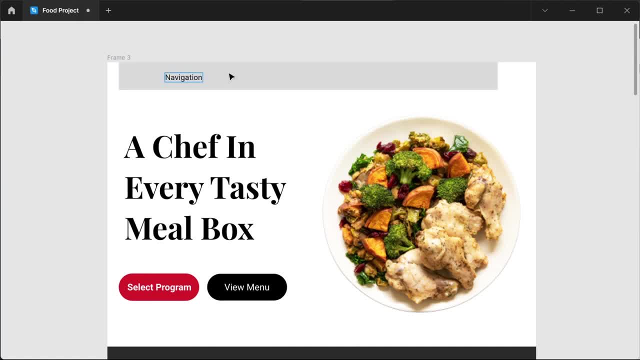 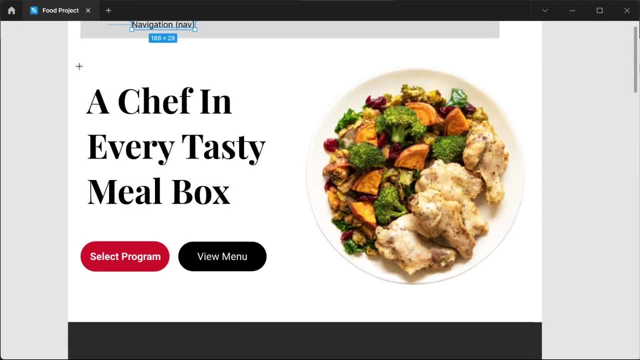 navigation. so for that we can use a nav tag. okay, so you don't have to worry about all of this. so you don't have to worry about all of this, so you don't have to worry about all of this crazy terminology. but i just kind of want to. 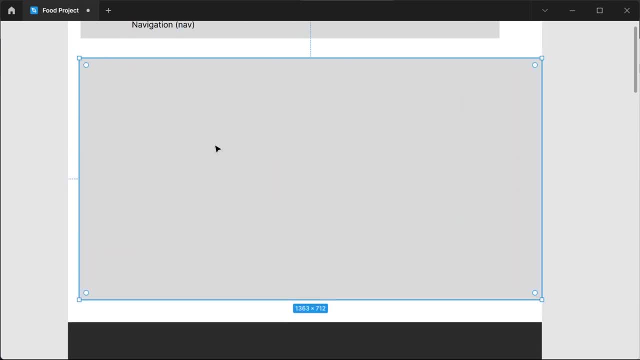 crazy terminology, but i just kind of want to crazy terminology, but i just kind of want to show you, show you, show you, and this will be our header area. so we and this will be our header area, so we and this will be our header area, so we can just write a content for here, like a 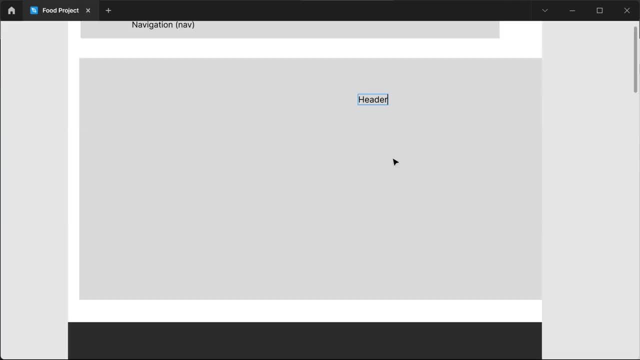 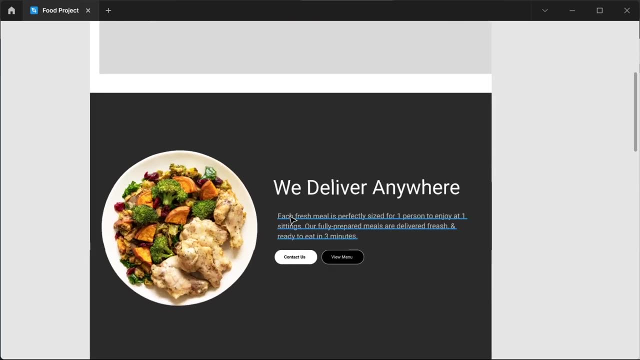 can just write a content for here like a header and let me just make that. oh my goodness, why am i opening the tab? uh, we have to make that bit bigger, like so. so this will be our header area and then this can be our section area, and 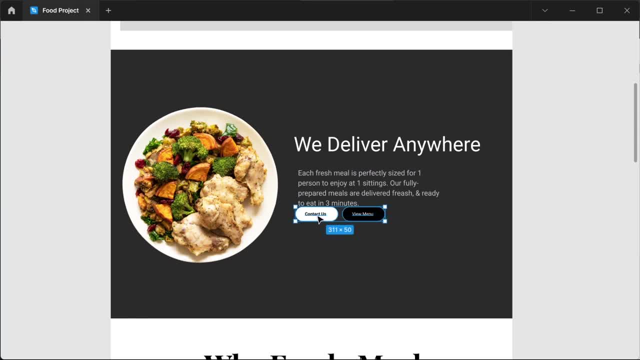 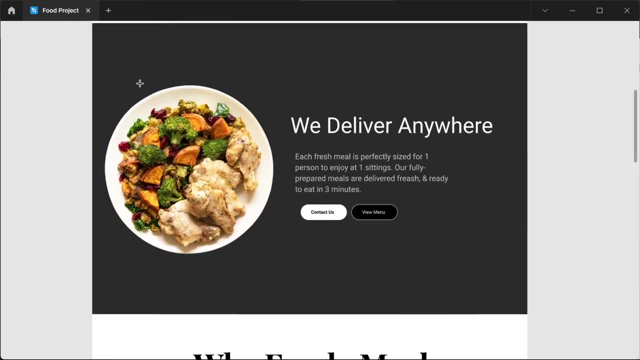 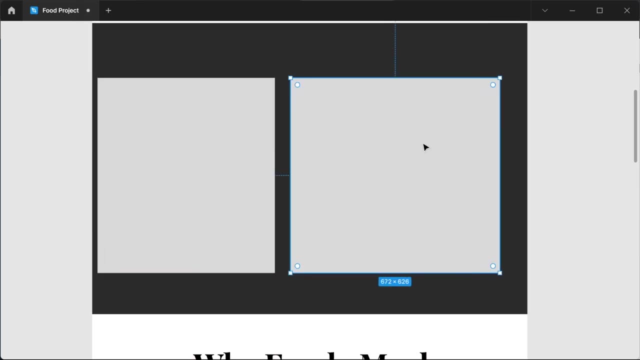 i know i was horrible back then. i didn't have that much skills on a ui ux, but now i do have a lot of skill. i have taken a lot of courses and stuff like that. so this will be maybe um section one and this one will be for maybe like a content section, so we can also just write an article in. 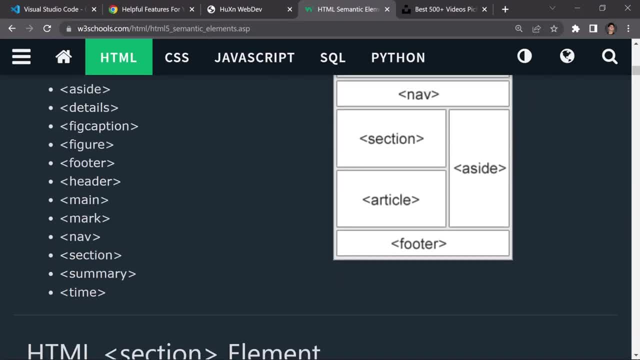 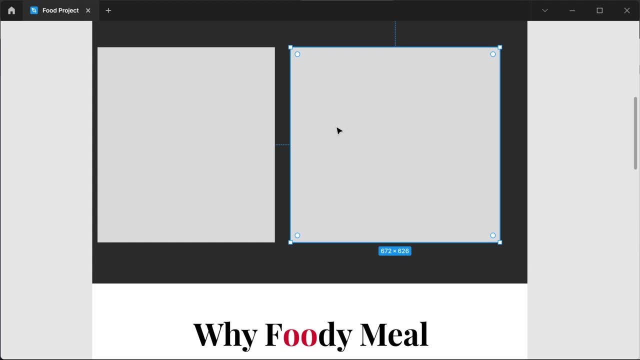 here. if you want to, we can use article section, which is this one. maybe let's show you this is article. we can also just write a detail section if you want to, because we are putting a lot of details in there and then we have. you know what. we are going to be using a detail section for this. 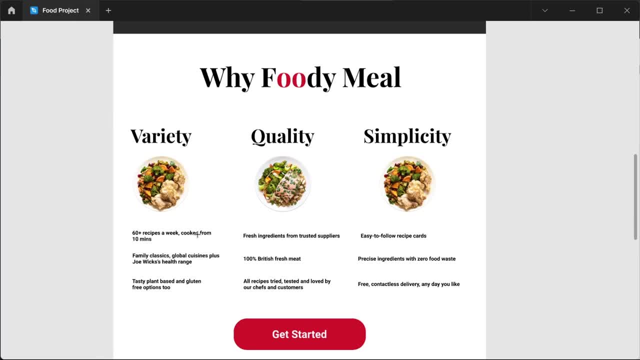 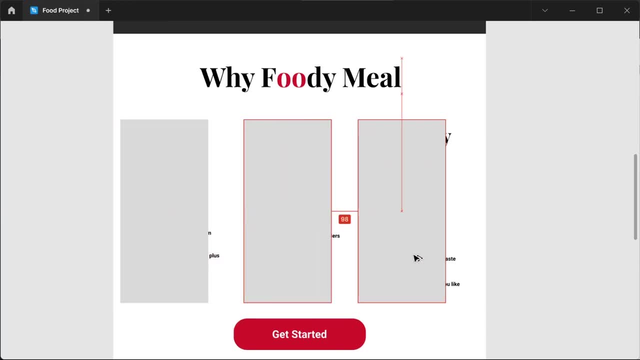 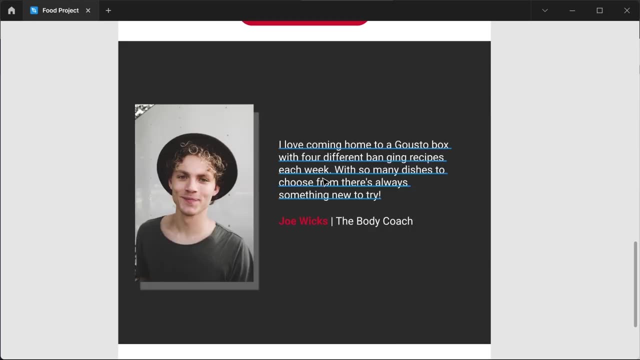 one, so let's just put, or you know what? this is going to be the first section. this is going to be what we can also use aside for that, if you want to. okay, so this is how it looks like, and the button will not take anything. and this is going to be it, for you know what? uh, section. 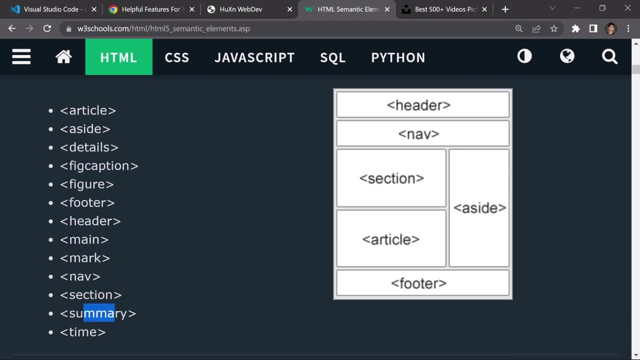 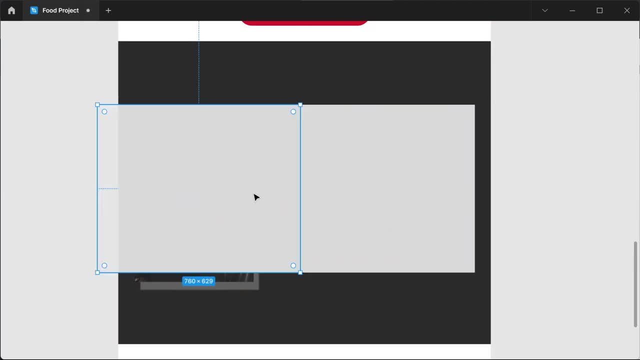 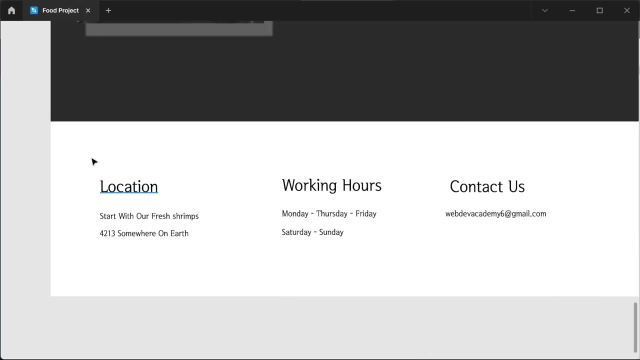 summary and stuff like that. uh, okay, so we can also put that as a detail section. so this is going to be the detail section and this one is going to be just a simple actual section. so we can just give a name if you want to, but i don't have that much time to show you everything. and finally we are. 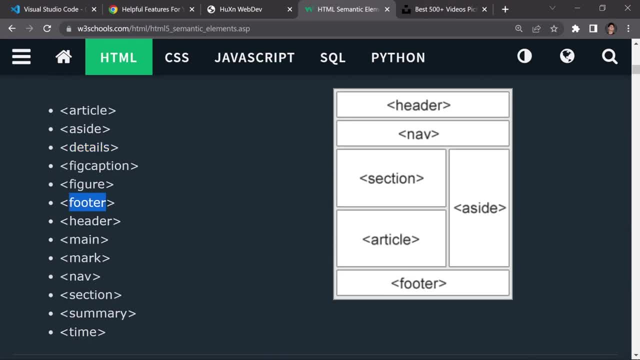 going to be adding a little bit of a detail section. so we are going to be adding a little bit of a detail section. so we are going to be adding a little bit of a detail section. so we are working with a footer and that. okay, so we do have that photo right here, so this area will be for 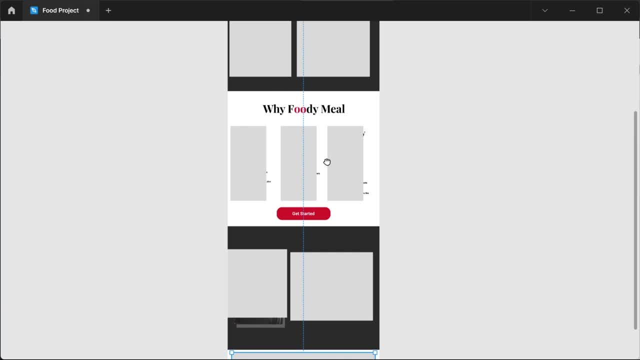 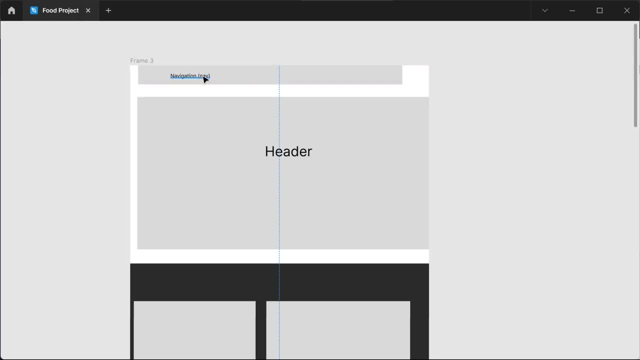 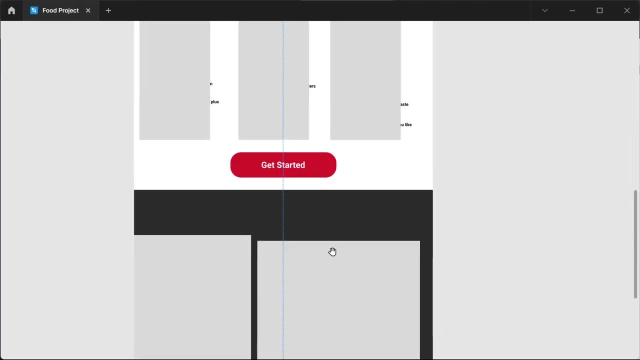 forward. so now, if you just zoom back and now here you can see, first of all, if you want to build this website, so we can either build this website by using a divs and span, or we can also just use like navigation header or yes section, like two section and detail section or three section. right here we. 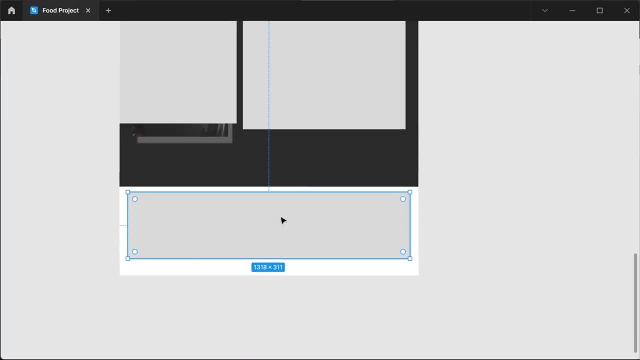 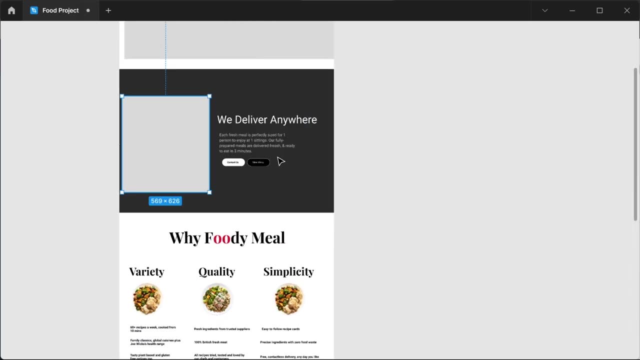 can also use article section and caption and stuff like that and finally we will have our folder. so this is just it. for a demonstration kind of purposes, like, we can use these elements, but if you don't want to use that, so you're totally free. like, if you don't want to use that, so you can use. 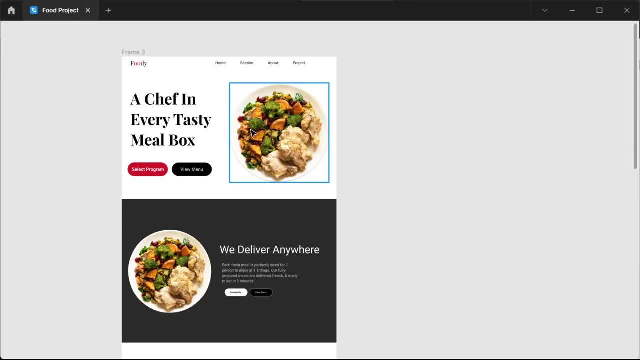 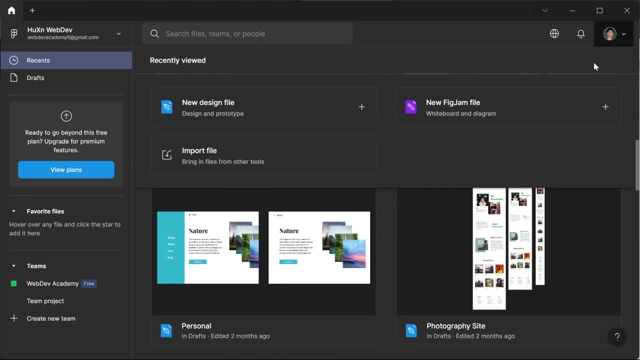 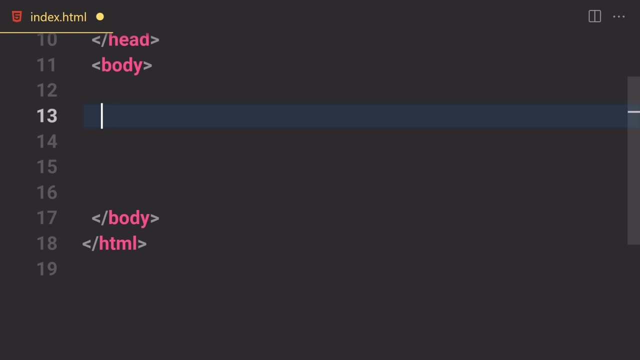 the other stuff, which is our divs and span. so now let me just show you how all of that will work and how all of that looks like. so you know, i'm going to close that one, and you know i'm going to close that one. i want to close also this figma file as well. we don't need that for now, so we have first. 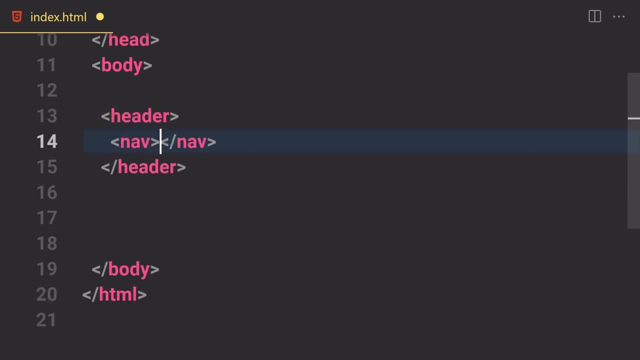 of all a header. so we have first of all a header. so we have first of all a header. so we have first a header. inside this header we can also write our navigation, and inside this navigation we can just write our ul, then li and then anchor tag and stuff like that. so this will be or kind of like a 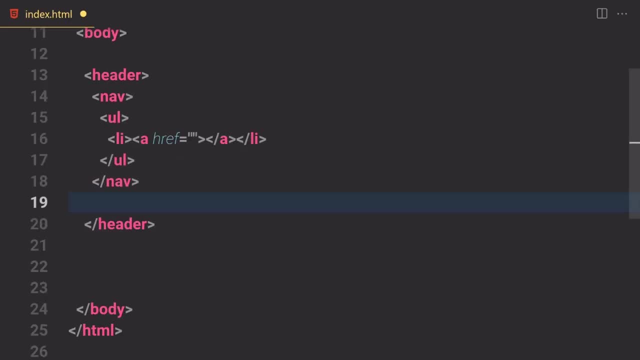 or navigation. you don't have to type this code, which i'm typing right now, but i just kind of want to show you just a quick preview of it. and then we have our section. inside this section, we can write a details section, because this is going to be your detail section. we can write our 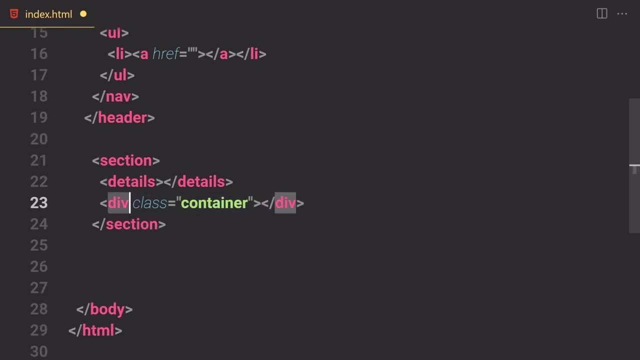 container, and here you can see i've already used this div right here. okay, so we can just replace every section, if you want to. so let me just write a section in here and we can also write article maybe. so i'm going to just write article and like article and we can. 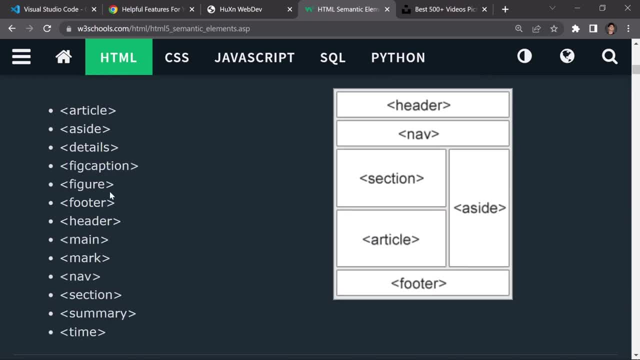 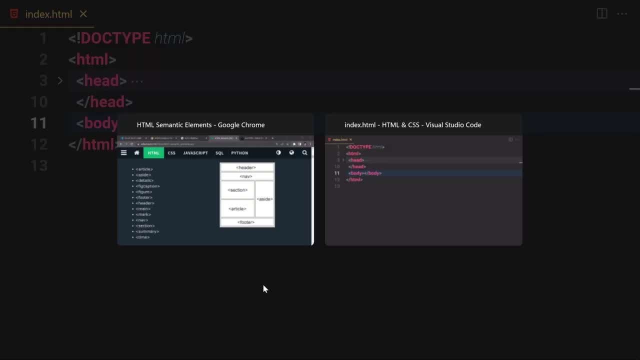 write. we can work with all of these kind of- uh semantic elements right now. so this is kind of a preview of our semantic elements and throughout the projects we are going to be using uh, all of these semantics element and we are going to be also using event span. i can't lie, i use this. 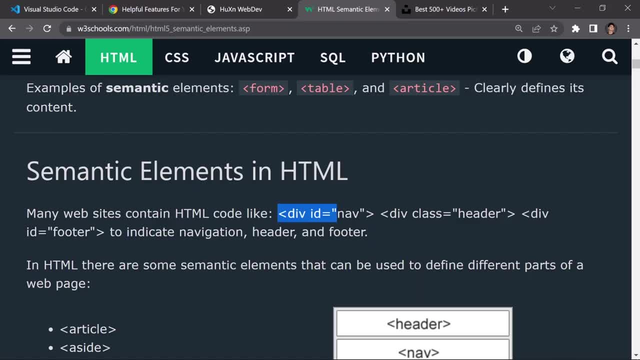 defense pen all the time and you will see that and i'm going to show you how to do that. so let's go ahead and open your guideе to see where you want to go. for example, let's say: uh, similar. okay, we are going to use an html file. i'm going to copy that over here and i'm going to say that this html 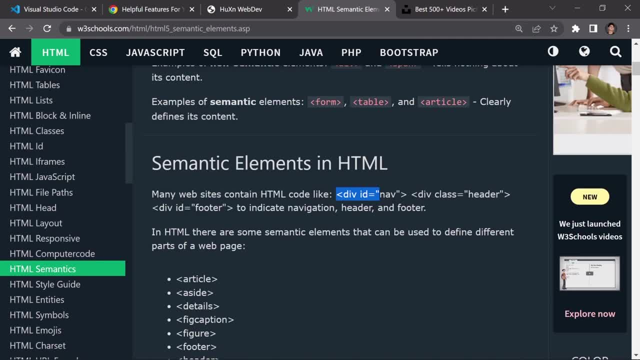 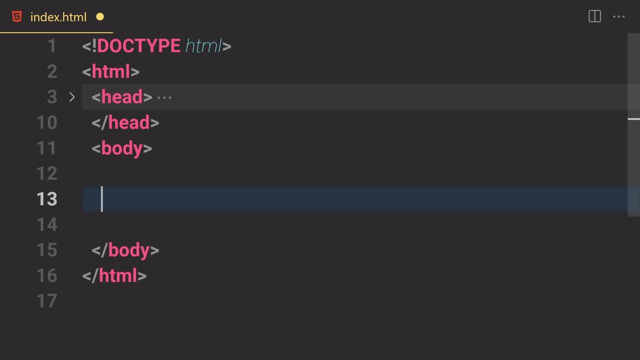 ok, save as my ads, wife. okay, okay, so online. uh, that's then. we are going to record the area as our web pages, as we have just done with the html archive object google tab, this page, this is basically our html grid, soですね, with which we use some assets for the html. 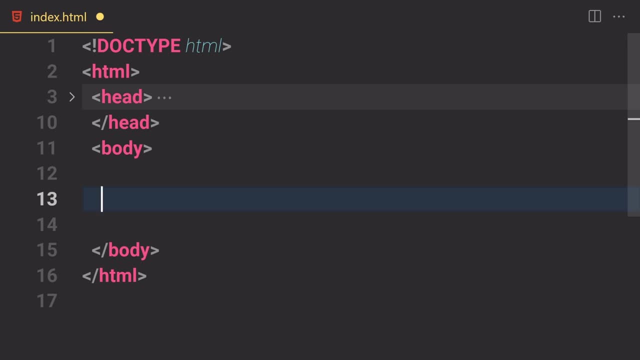 so you can see we are going to copy each other options and then we're going to use every cái data as a title. because you want a couple of lawyers, we can also do the видел eventually in a different way, ever in in other ways. so that is in addition to all the html sites. 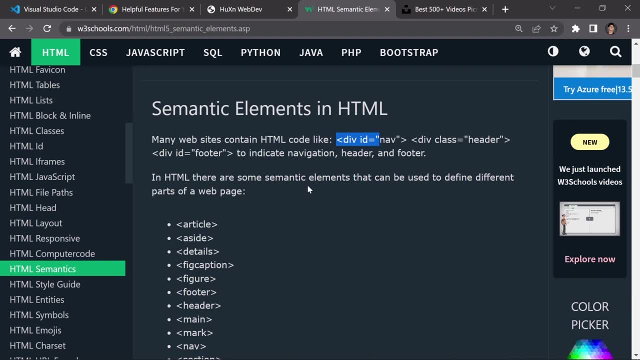 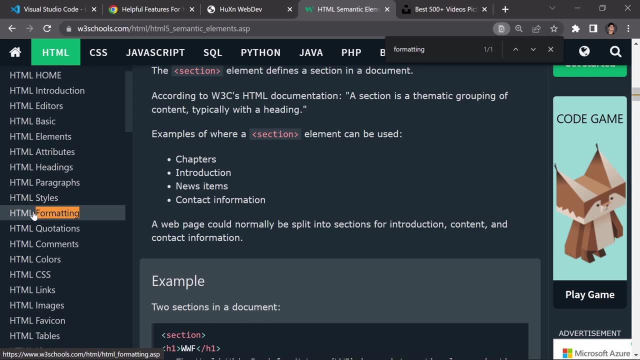 semantics, but uh, typography. first of all, we just have to hit control and hits uh f, and here we just have to write formatting, and here you can see we are now getting this html formatting right here. so if you click on that, so it will now brings us to that html formatting web page. okay, so it's. 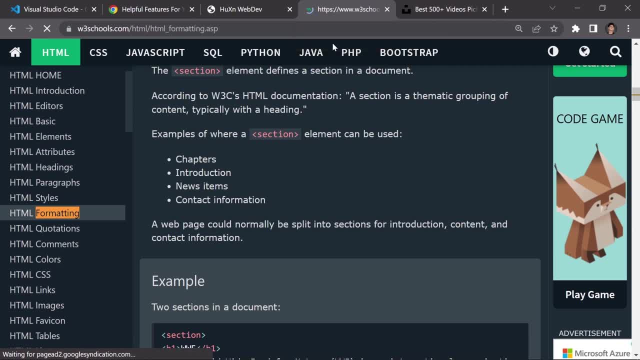 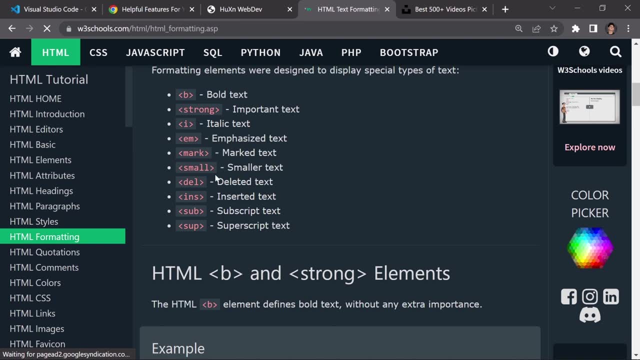 taking time. you know what it will render. yeah, it's taking a bit of time, okay, so now it's back. so we have all of these kind of typography related html elements right here. so we have b for bold and we have strong, and strong will also make our text bolder. and then we have i for italic, and then 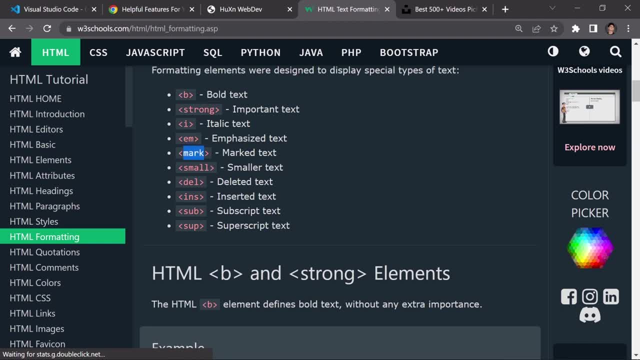 emphasis will also make our text italic. then we have a mark and it will just mark our text. then we have small. it will be just a little bit smaller than a paragraph. then we have a del, as the name suggests, that it will allows us to line through our element and it will look like kind of like. 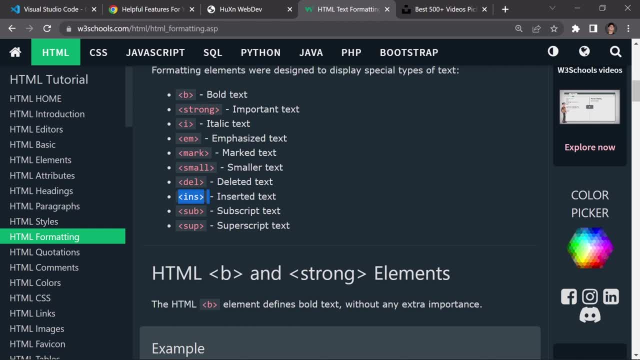 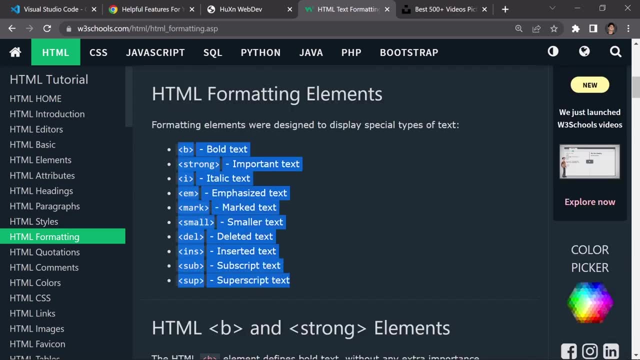 a deletion of the elements, and then we have inserted, we have um, superset and subs. i mean like subscript and we have a superscript. so now let's see what we have here. so we have a subscript and we have a superscript. so now let's just learn all about that. so first of all, we are going to be starting from b tags, so i'm going 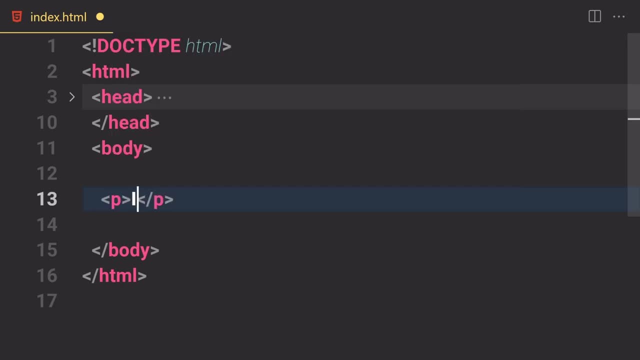 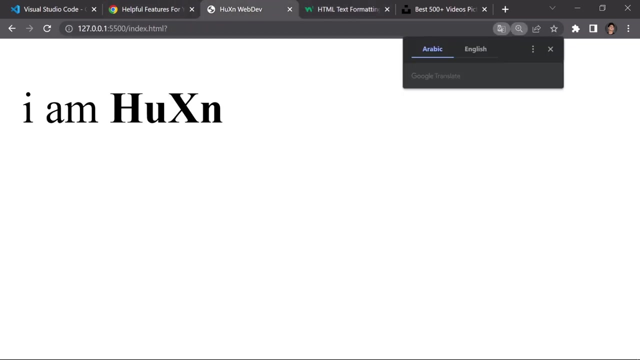 to just write first of all a paragraph: um, maybe i am, uh, yeah, i'm going to just write lowercase i am- and then b, and here i'm going to just write my own name, huzzain, and it will be now bold. so if you save that and if you check it out, so here you can see this huzzain is not only bold, that's because 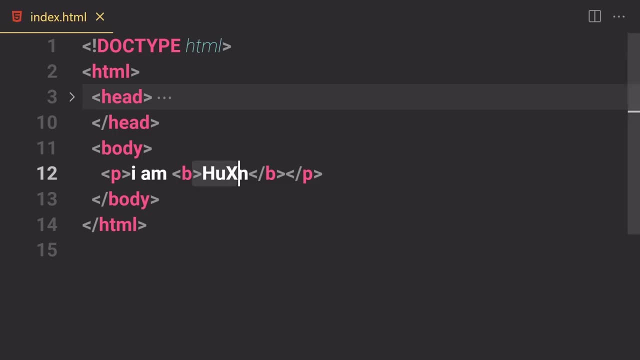 we put that inside a bold tag, like a b tag, and we can also use a strong tag for that instead of writing b. so we can also just use a strong. so i'm going to just replace that with strong and if you save that and boom, okay, so we are now getting this strong tag right here. i mean like that boldness. 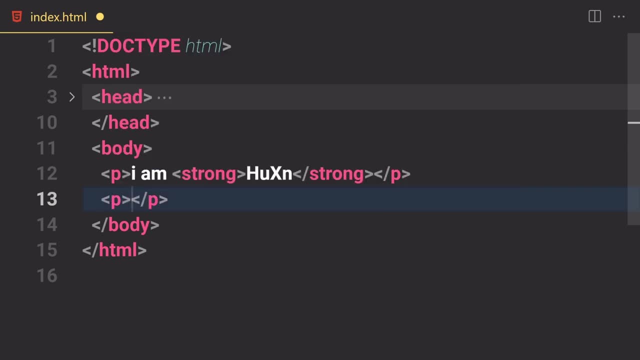 now, the next thing which you have to learn is that paragraph: i am, yeah, i'm going to just write like i am, and then i, and here i'm going to just put my name of huzzain, and if you save that, so what are we getting here? you can see the difference. like this one will be italic and we can also italic. 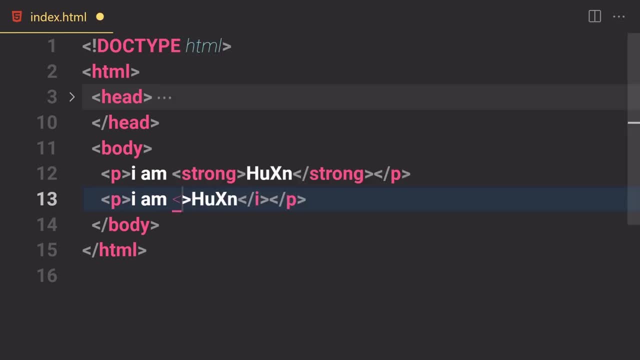 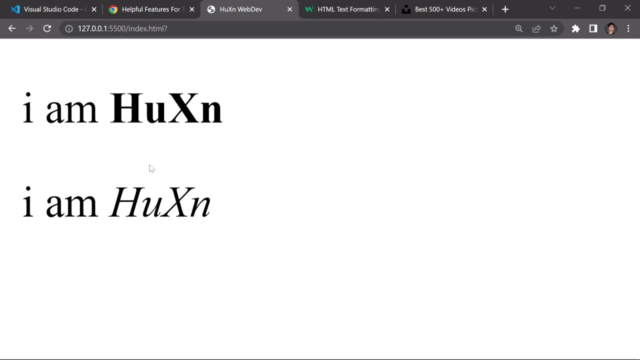 there by using em for that instead of writing b. so we can also just write like i am, and then i am writing i, so em stand for the emphasis, so you can just write em for that. and if you save that and boom, here you can see, both of them will be the same. like i will do the same thing. like it will. 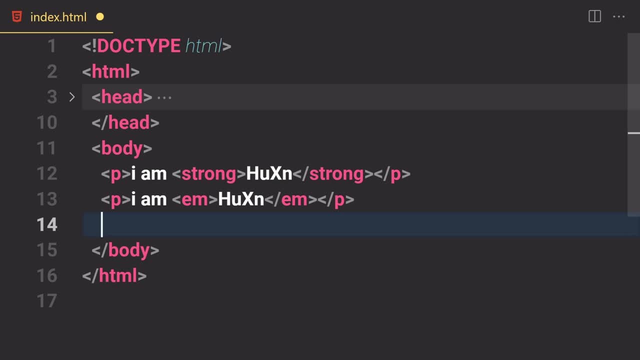 make it italic, and so will m okay. so now the next thing which we have to learn is something called a small tag. but before i do here, i'm going to just write like hello inside this, and i'm going to also put that hello in a small text. so instead of writing p, we have to write small right here. 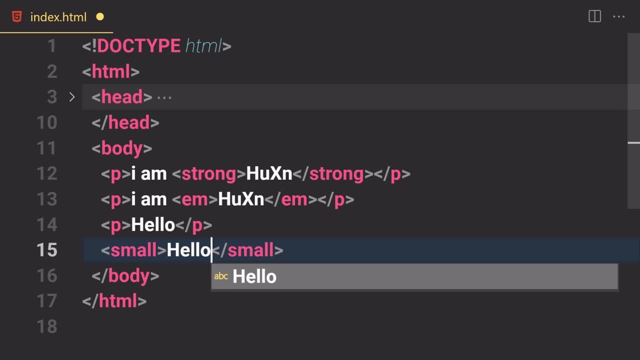 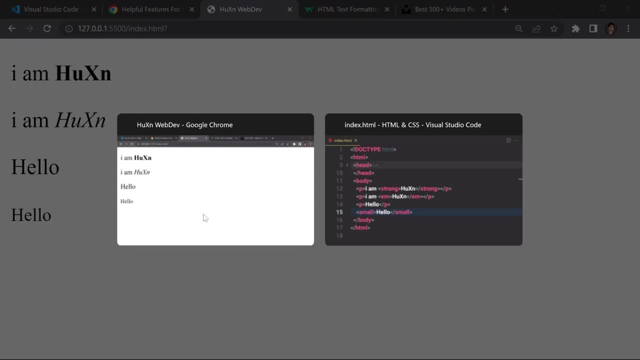 and i'm going to also put a hello in there, so it will just give you a little bit of difference. so save that, and here you can see, this small is just a little bit smaller than this hello one right here. okay, so this is how it will look like. now let's just 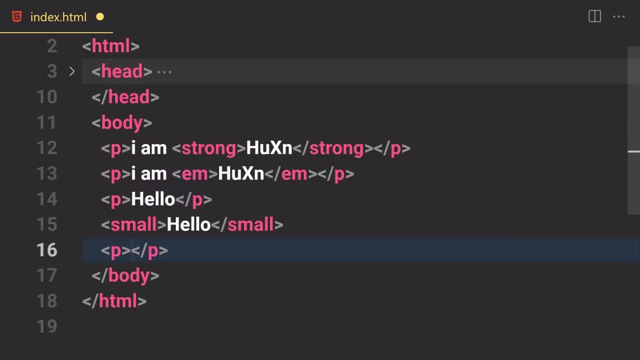 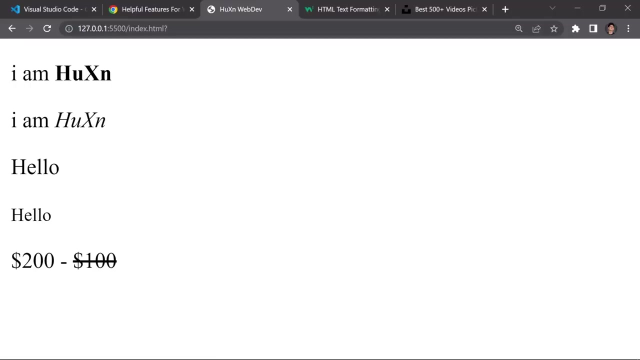 learn about their deal. so i'm going to just write like paragraph and the price used to be like two hundred dollars and now the price is just deal. let's just write deal in here, and now let's just write hundred, um dollars, and if you sell that, so the price okay. so we messed it up right here. 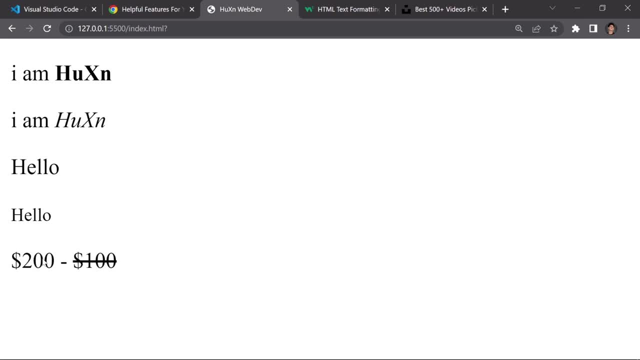 the price used to be a hundred dollars and now it's two hundred dollars. you know what i'm going to change: this one to two hundred dollars and this one to one hundred dollar if we sell that. and this is how we can use that deal. and we can also just write a paragraph: uh, and here we can. 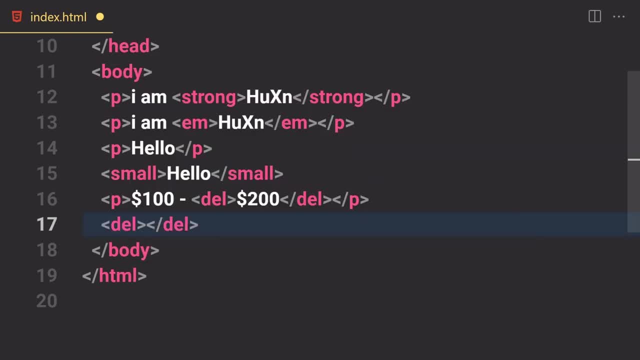 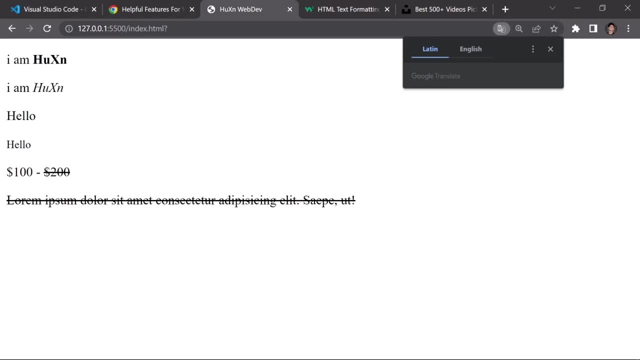 just use our deal or not even a paragraph. we can just simply use a dell and here we can just write a lorem ipsum if you want to like lorem 10 and save that and boom. okay, so it will just line through our element. okay, so we can also. 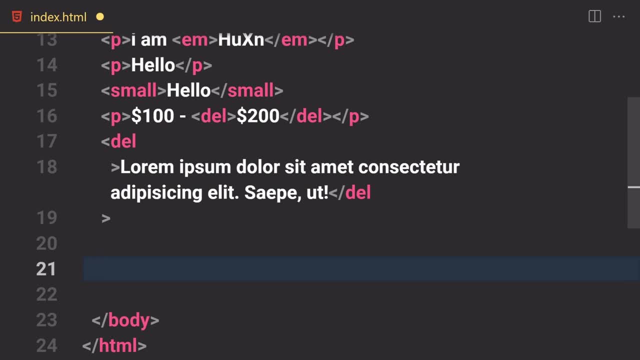 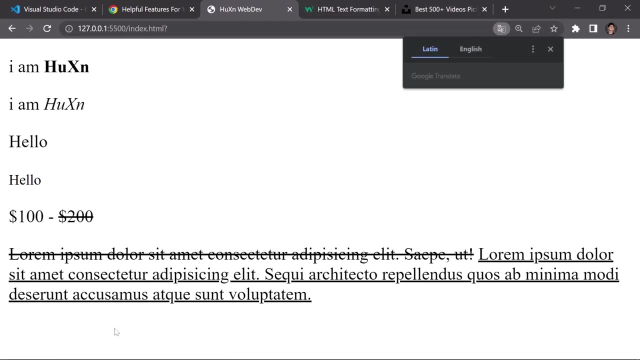 achieve the same result by using a css, but you know what we are learning about html, so we don't have to go into that much details. so we also have a ins- this is the alternative for that- or del one, so we can just write like um lorem of maybe 20.. so if you sell that and here you can see it will. 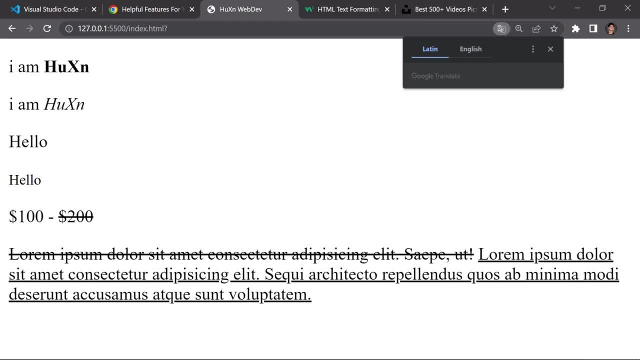 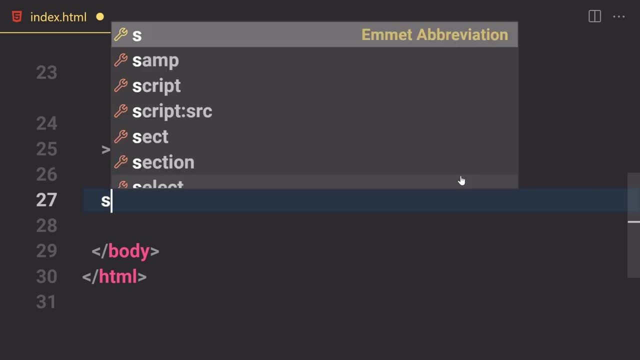 just gives us a line underneath the text, right here, so it will now gives us a line at the middle of the text, and it will now give us a line underneath the text, right here, so you can see the differences between both of them. and now let's just learn about a new one, which is called a subset and a super set. and then let me. 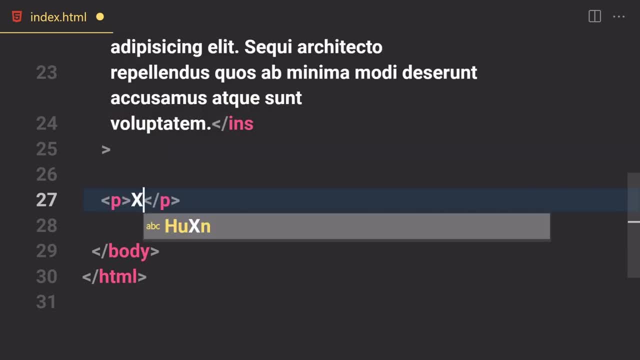 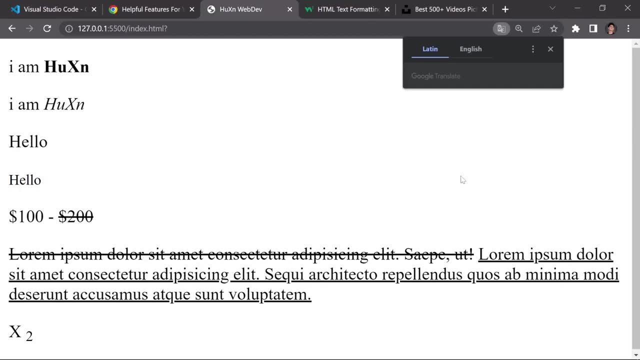 just write a sub in here, you know what? first of all, let me just write a paragraph and put our X in there. and now let me just write or, sub4, sub, and I'm going to just put two in there. so if you sell that, and what are we getting? first of all, let me just remove all of this coding from here. 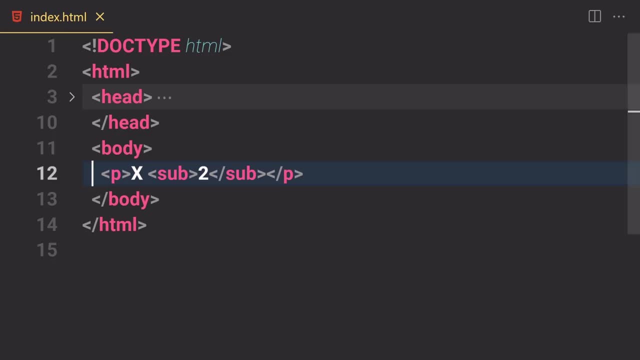 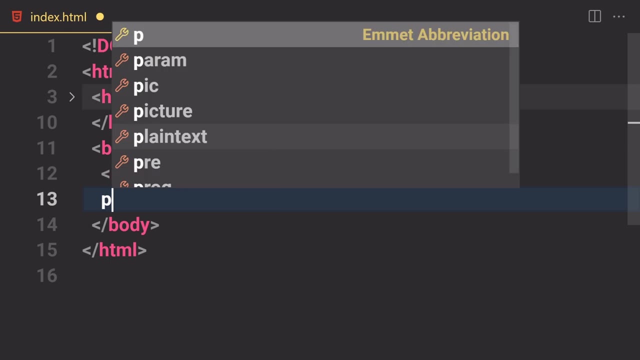 so you guys can see everything, save it. and now what are we getting? we are getting X, and then I don't know what you call that, but we have two. okay, so we can also write a powers, if you want to. we have to just write X and instead of writing a. 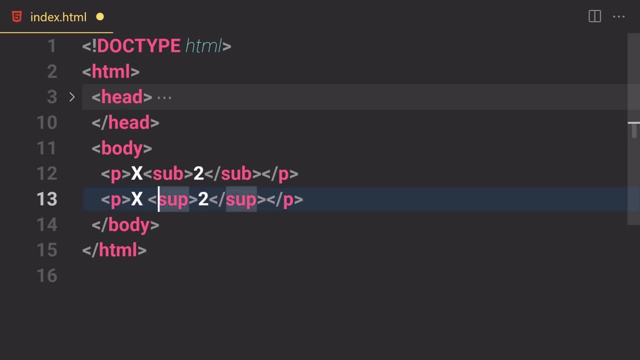 subset. we can also write super set like just a power of X. so if you just sell that and here you can see we are now getting results like this, so we can also write instead of writing. two, we can write a gibberish in here if you want to, and this is how the gibberish will look like and we can. 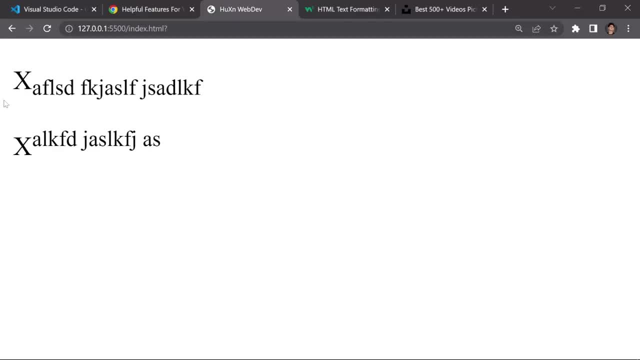 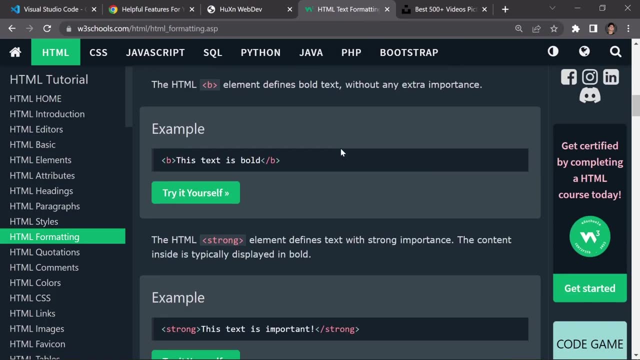 also put a lot of gibberish in here and if you sell that and this is how all of their gibberish will look like, so we can do crazier stuff like that. so these are just a little bit of typography related uh tags right here, and there are a lot. 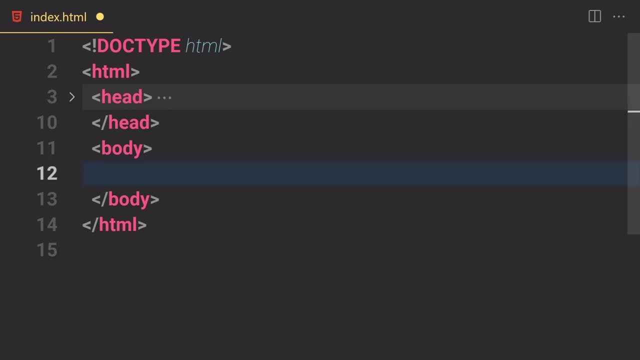 of typography related, so we can also use a mark. I'm just coming up with ideas, so I'm going to write like paragraph. you will only fail when you stop trying. and now, if I want to just like mark this last word and I want to just put that in a mark, okay, so we have to first of all write a mark. 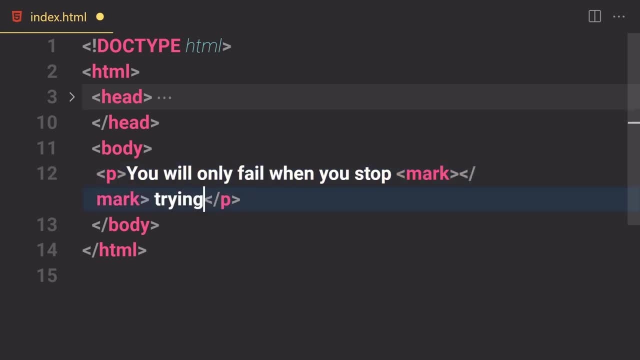 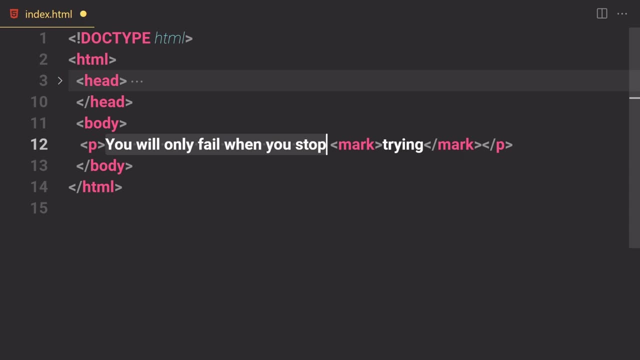 opening tag and then mark closing tag, and I'm going to cut this thing from there and I'm going to put it inside a mark. so I'm going to zoom out of it and this is how it looks, like like you will only fail once or when you will only fail when you stop trying. so if 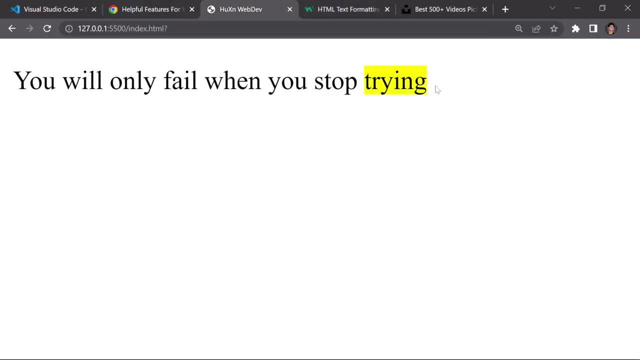 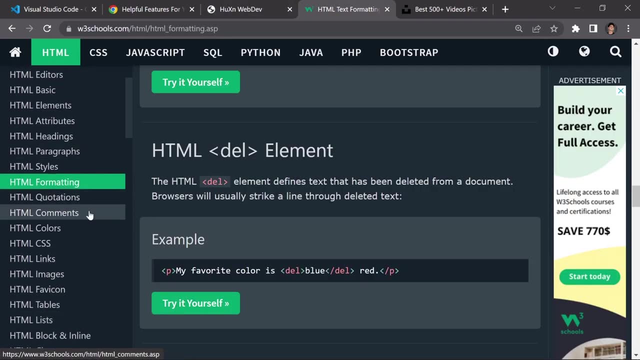 you sell that and if you preview it, so here you can see, it will now just highlight it right here. okay, and there are a lot of them if you want to like learn more about these typography related kind of HTML elements so you can learn more about that. you can also write a quotation if you want to. 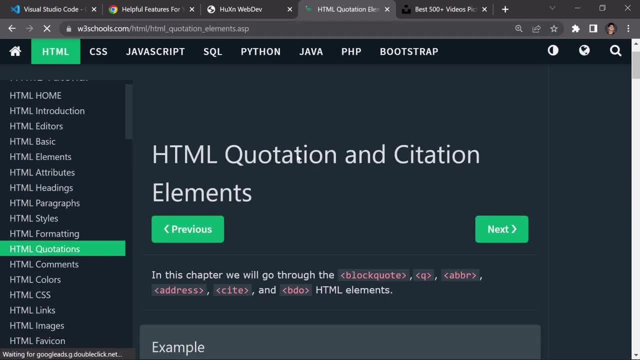 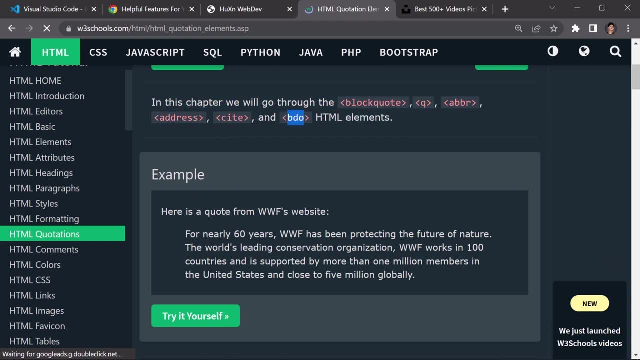 so I'll just click through all of them, because my internet connection is extremely low. I don't know what's happening to it. we can do citation. we can provide addresses, we can do. I don't know what's that even stand for. so suppose if you want to get a quote, so if you want. 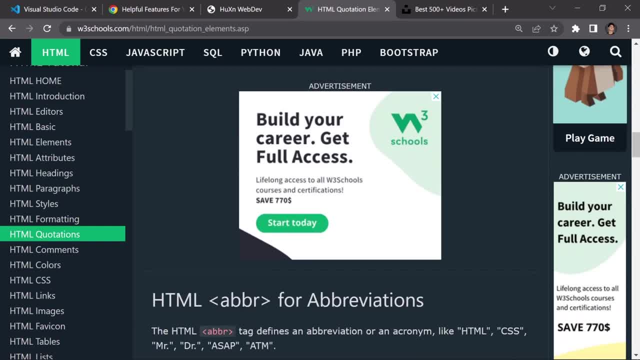 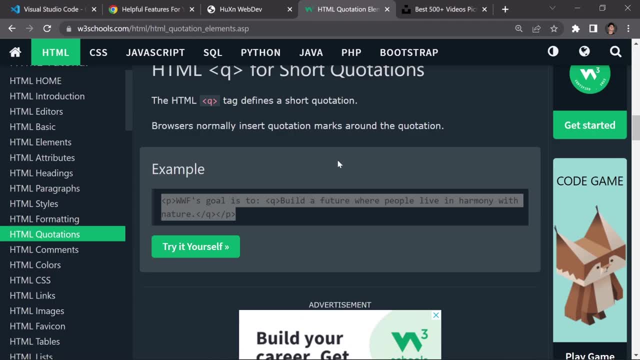 to work with a quote, so you can also just write a quote, and also I also forgot to include one more. but you know what? first of all, let's just copy this text code and I'm going to paste it right here, and if you save that, and here you can see, it will now just provide this quotation right here. 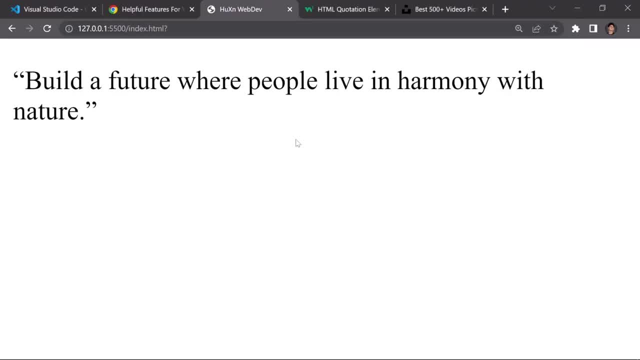 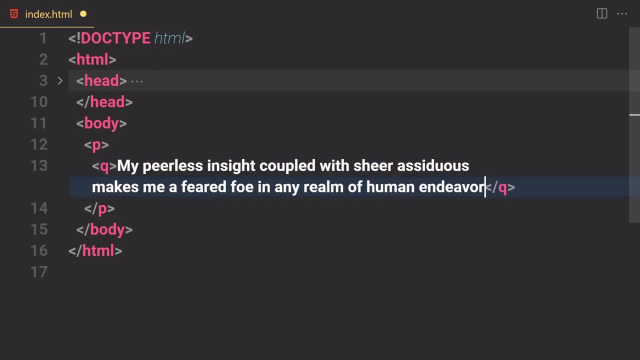 so I'm going to just remove that and replace it with the andrew state father quote. real quick, i'm going to replace this quote to andrew's father quote, which i really like, so i'm going to just save that and here you can see it. 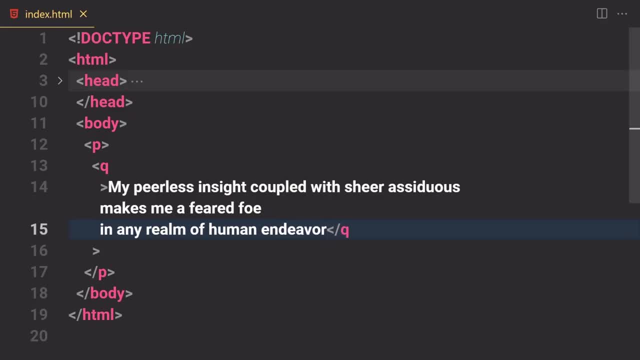 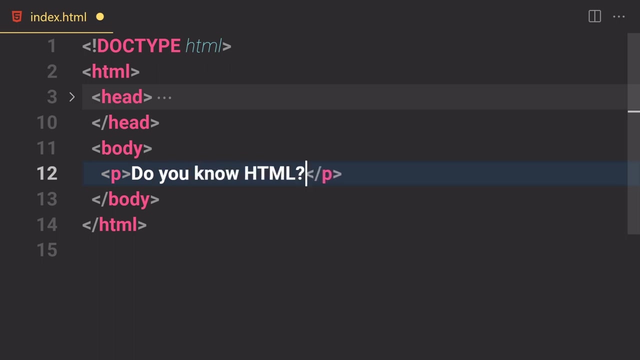 will now gives us this quotation right here. okay, so these are quotation, but my favorite thing which i want to show you is something called abbr tag. i'm going to zoom in a bit. first of all, let me just write a paragraph and do you know html? okay, so you know, i'm going to put that in abbr tag. 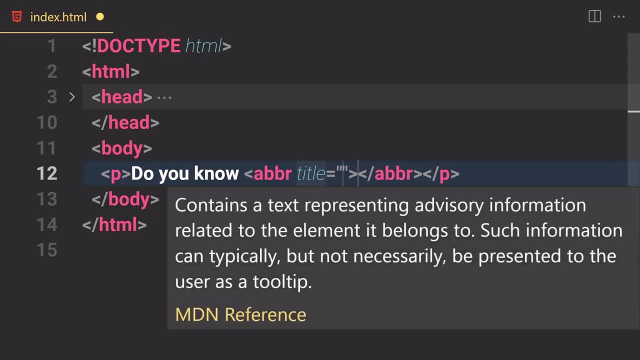 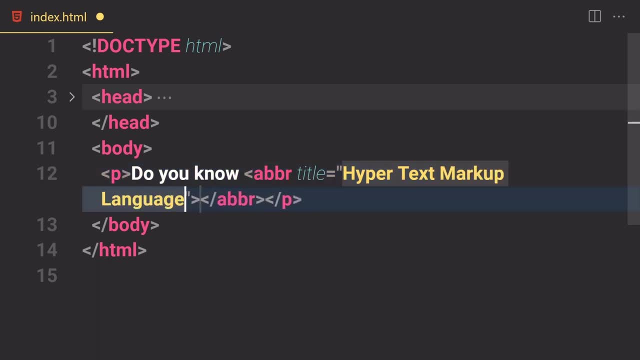 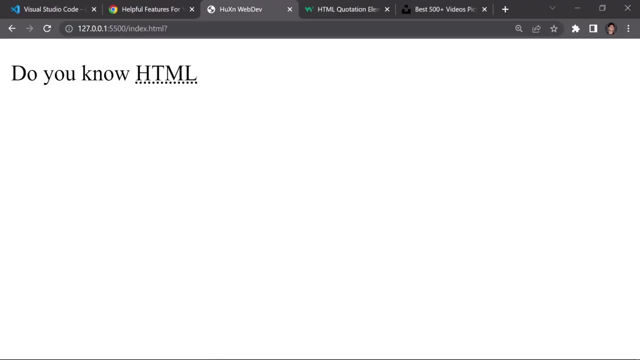 and, as the name suggests, there it will be abbreviation text. so here we just have to put our title, so html just stand for like hyper tags, mark up language, okay, zoom out of it. and here we just have to put our html in there. and if we save that and here you can see, do you know html? and 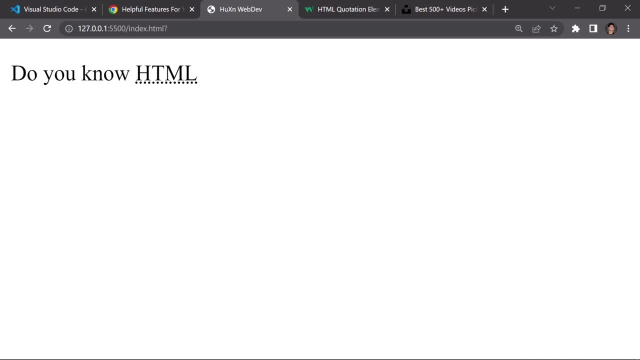 here you can also see these dots. but if i hold down that andrew state father quote andrew state- my mouse over to it. so what are we getting? we are now getting a hypertext markup language right here if i hover my mouse over to this anchor tag- not anchor, but this uh, simple content right here and 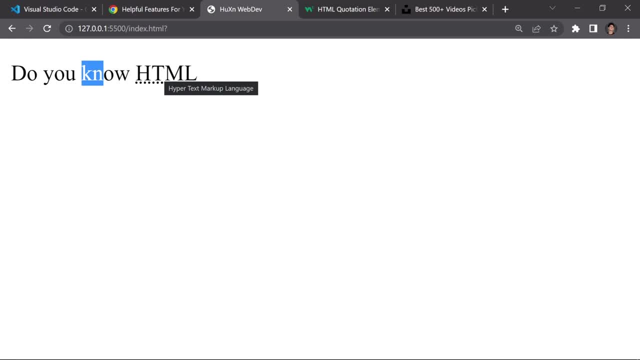 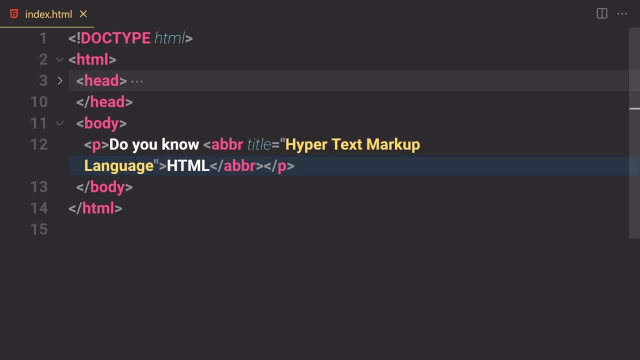 here you can see nothing is happening. so if i hover my mouse over to this html, so it will not give us like hypertext markup and language. so if you click on that, nothing will happen. so this is why i really like abbr. it can be useful in some situation so you can learn more about this. 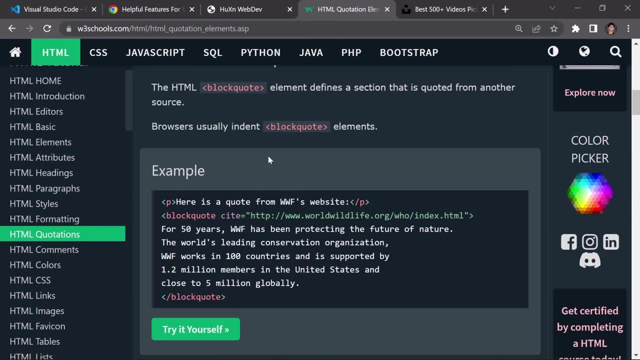 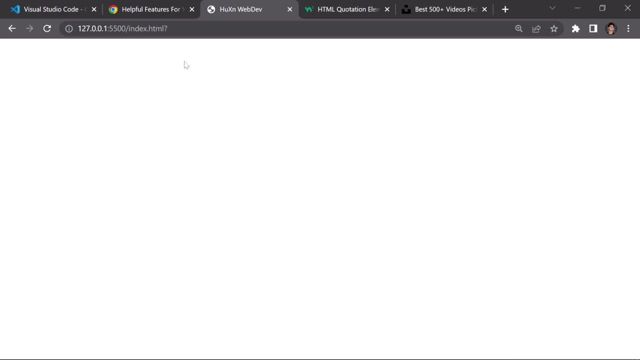 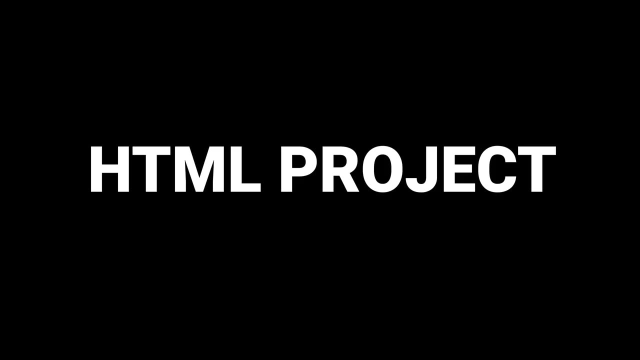 quotation and these hair typography related elements if you want to. but i don't want to waste your time and my time because we are going to be doing a lot of crazy typography once we jump into a css. but for now, i guess that would be it for html. okay, so you know what? let's just 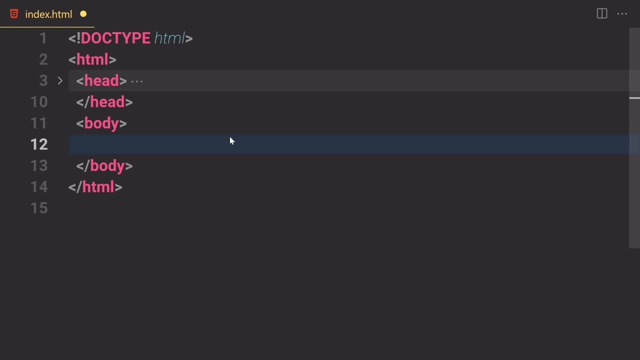 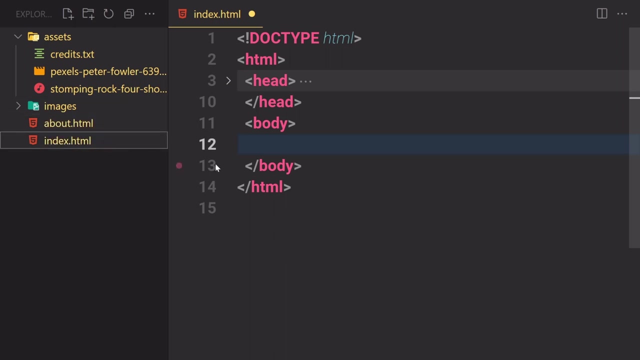 start working on a project. first of all, we are going to be building a portfolio project using just a pure html, not anything else. i'm going to just delete everything. i'm going to highlight everything and boom, everything should go away except that images. so i'm going to just select that as well. you know what? first of all, let's. 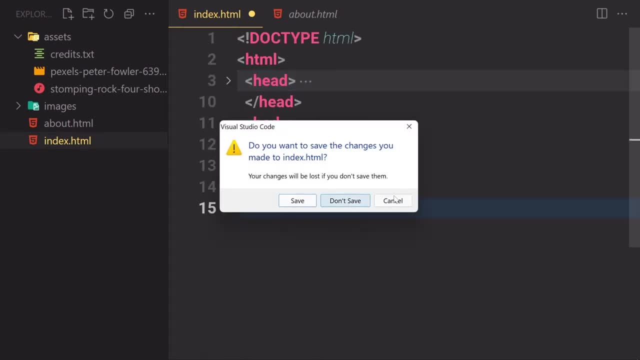 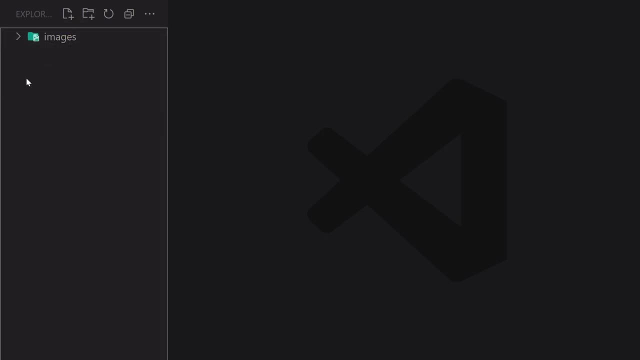 just shut down our live server and i guess that would be fine cell file. let's just remove both of these files and also this assets folder. so currently we are just having this empty folder with one images folder and we just have that one images. so i'm going to just drag it out, i'm going 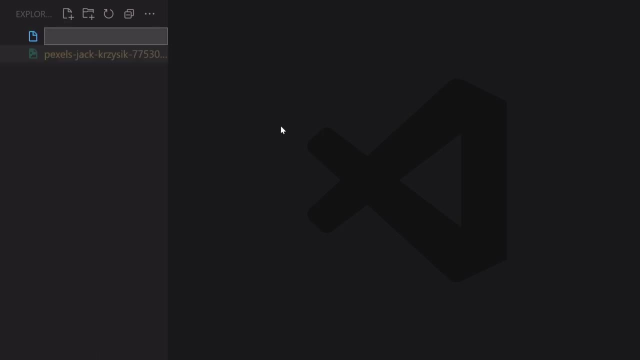 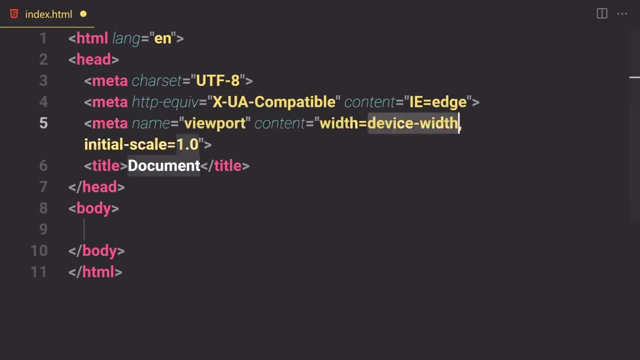 to also remove this images folder. and now let's just start working on our project. so anytime you want to work with html projects. so first of all we just have to create some sort of html file and inside that we are going to be using a image. so we have. 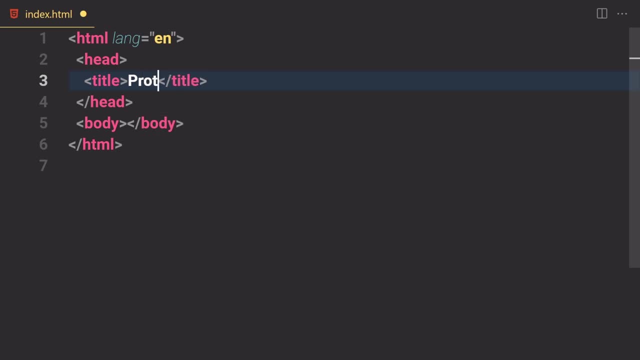 this structure of their html, so i'm going to just write: port all your portfolio project using html. that's going to be awesome one. i'm going to zoom in a bit and now let's just start working on, or maybe navigation, so we have our nav inside this. now we are going to have a lot of ul and alloys, so 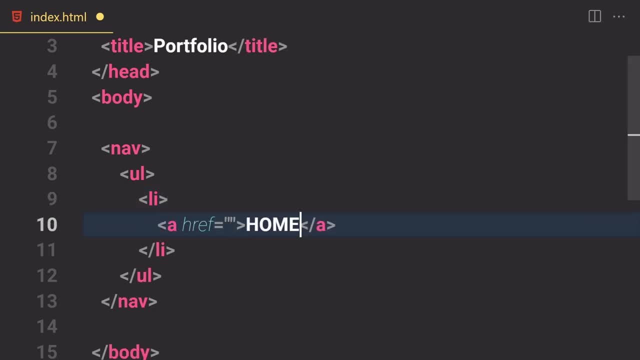 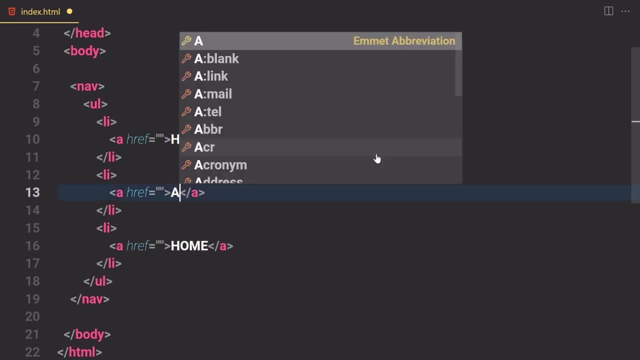 in each ally we are going to have or home, maybe. so i'm going to just write home and i'm going to duplicate this line, of course, for now. so zoom out of it. we have a home, then we have a bound section, and then we have or contact section. so let's just duplicate that one more time. 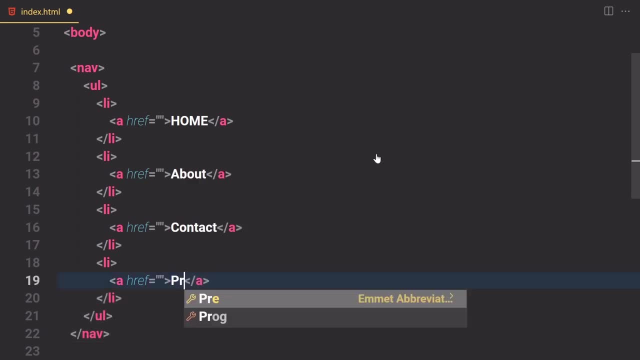 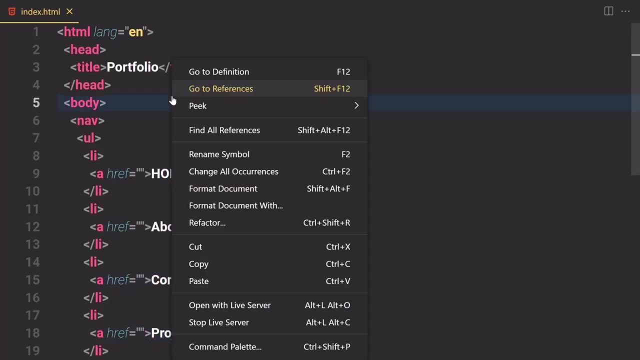 or what for a project section. so let me just write a projects in here, and knife is our file and i don't know what's happening. okay, so we're going to launch that in a live server, have to right click on it and then click on open with live server so that we can work. 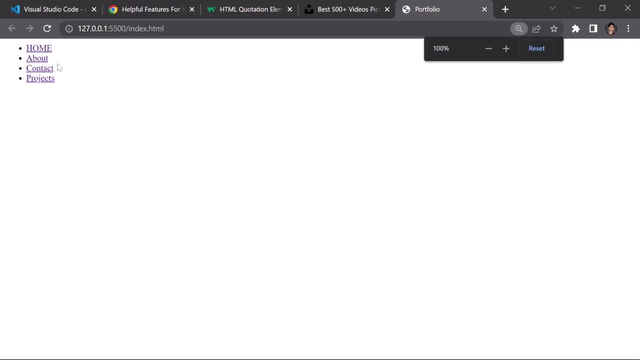 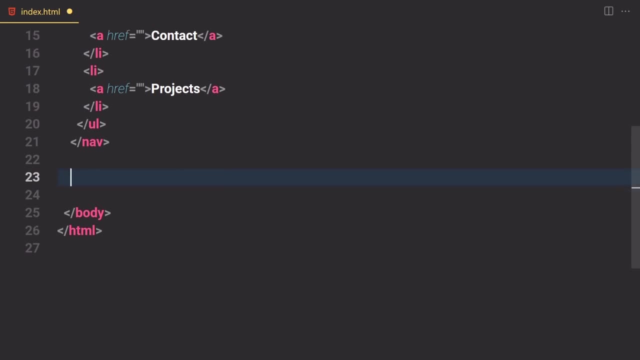 on that and here you can see we are now getting our first navigation right here. okay, so now we are totally done with the navigation. now let's just start working on our header area, or you can also call it a hero area, or you can also call it a main area, because 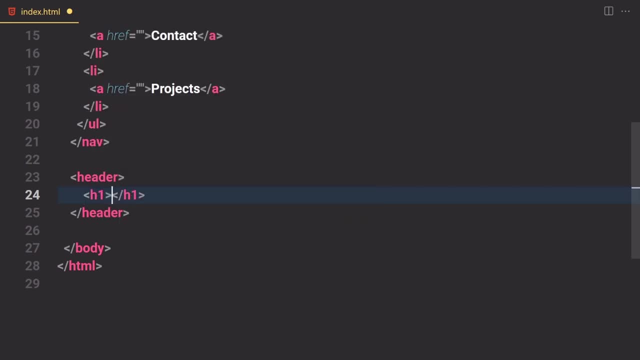 we are going to be putting all of our content inside this uh header area, so let's just write our h1. i'm going to put my name in there. you can put your name. if you want to, then let's just write uh to my personal part or audio right here, so that- and here you can see- we have welcome to my. 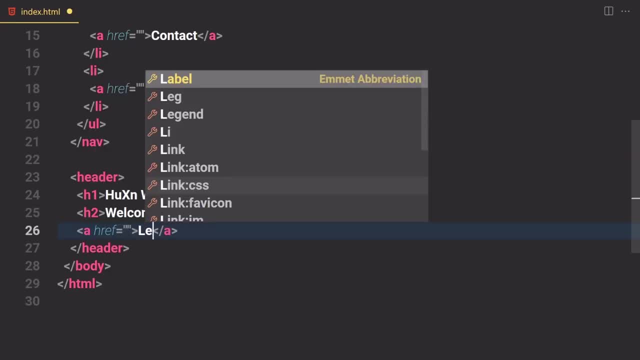 personal portfolio. let's just write an anchor tag. it will say: learn more. and if you sell that, we are now getting this button right here, kind of a grace button- not a grace, but an anchor button. now let me just write a section in that. and now, here we are going to be rendering our image. 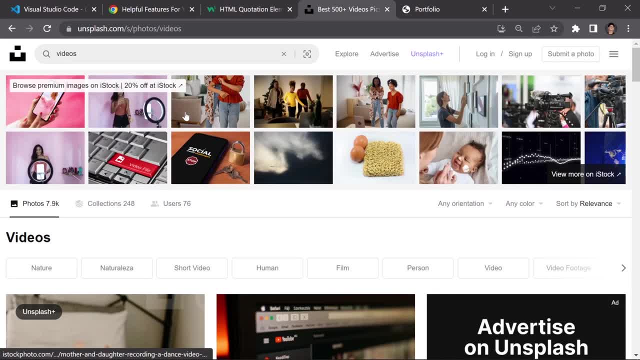 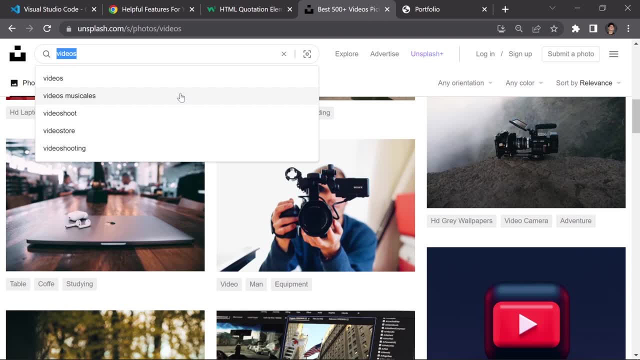 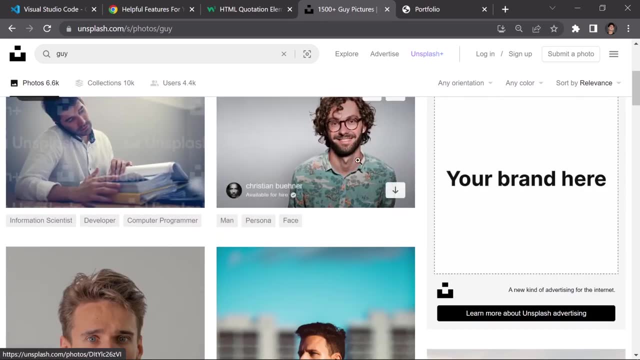 which is, you know what? we have to search for some cool guy. because i'm a cool guy, i'm gonna have to put a cool image of myself, so maybe um guy would be fine, i'm gonna just search for a guy. yeah, i'm totally nerd like this guy. sorry, i apologize, it's not, he's not a nerd, he's. 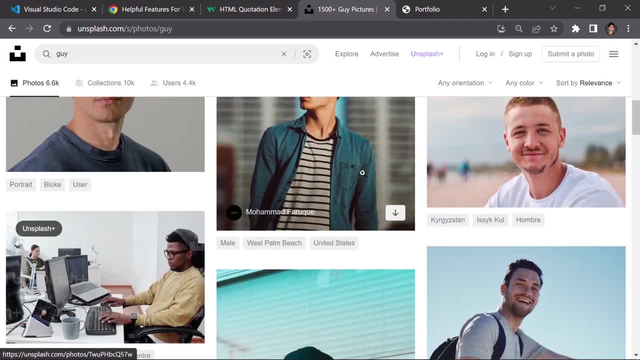 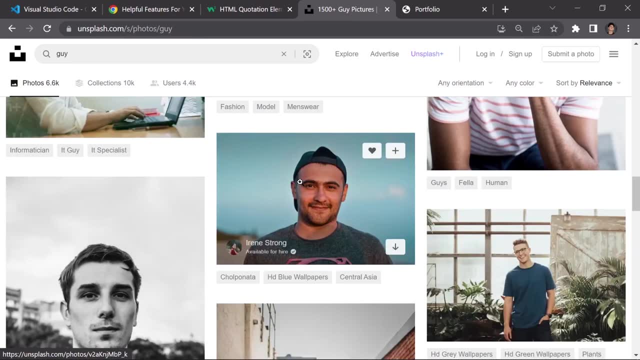 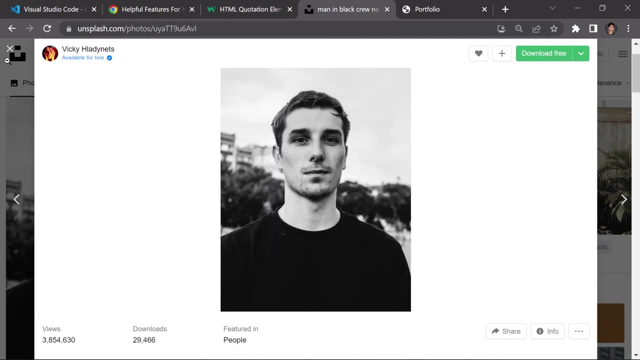 awesome looking man and i'm not like that much rude like the one. this image, uh, okay, so i'm gonna just search for some cool coin. i really like kind of these great colored images, so i'm going to just select professional shorts. i'm going to just copy this sky image address: 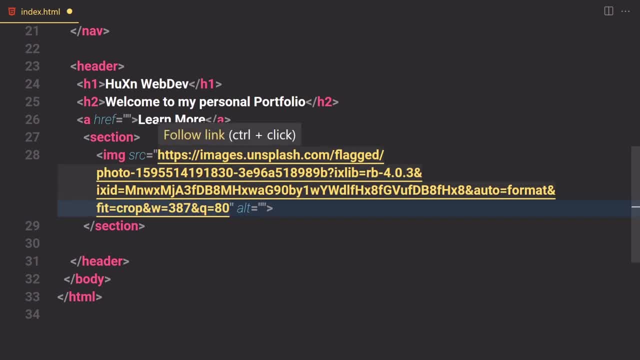 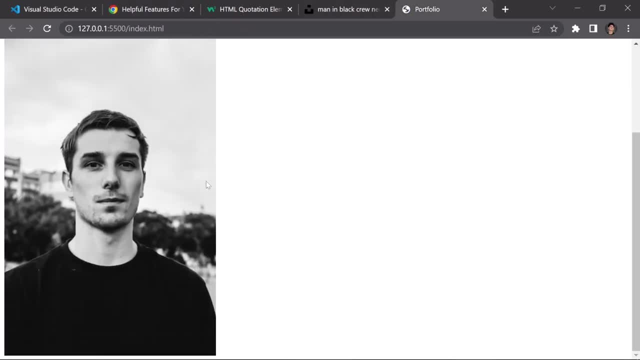 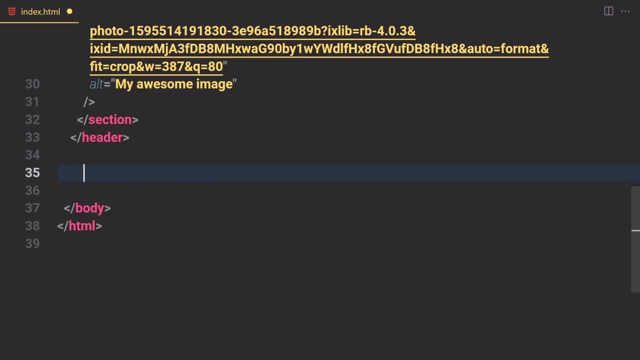 and now i'm going to put that inside. there and here we are going to be writing my awesome image, awesome image and cell file and boom, here you can see we are now getting our images right here and now. what else do we have to do underneath this section, or not even a section underneath this? 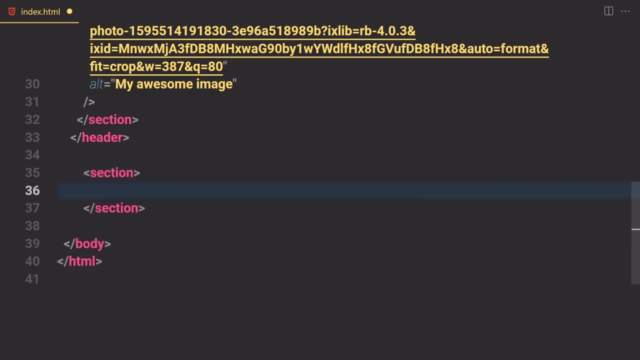 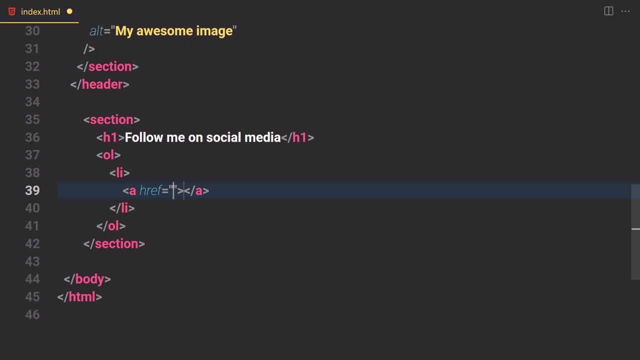 header. we have to create a new section and now inside this section, we are going to be writing h1 of follow me on social media. and if you want to follow me on social media, here are all of my social media. i'm going to just fast forward these social media because i'm going to have to copy all of my social media. 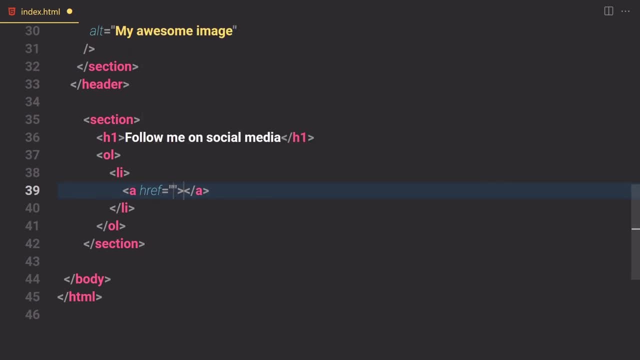 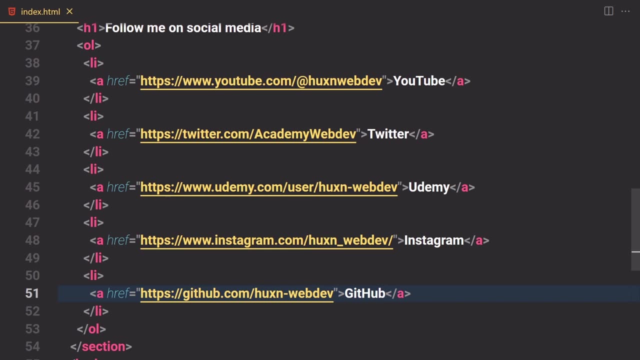 links and i'm going to paste it in here. and if you have your own, so you can also paste it in here. so i'll just see you in a second. all right, guys. so we are back and i just passed all of my social media links right here, if you want to follow me on youtube. so here's the. 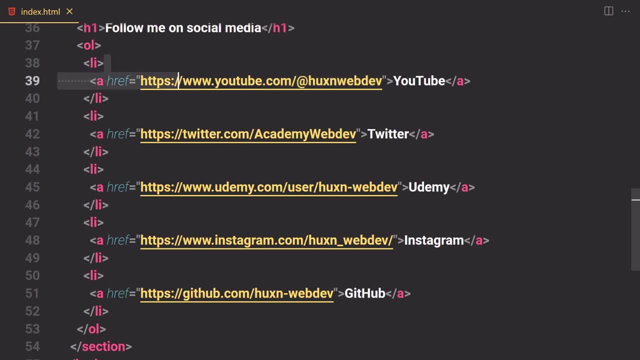 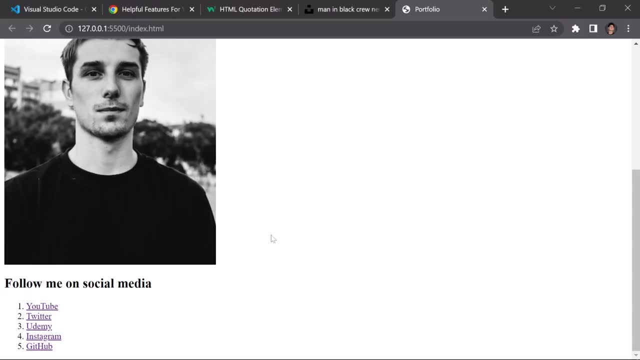 link, then twitter, then udemy, then instagram. if you don't want to follow me in any of them, so don't, but i will request you to follow me on github because i really love github anyway. so if you don't know what a github is, i have entire course on that if you want to check. 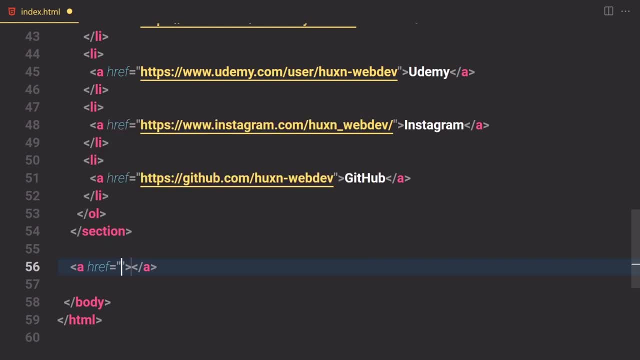 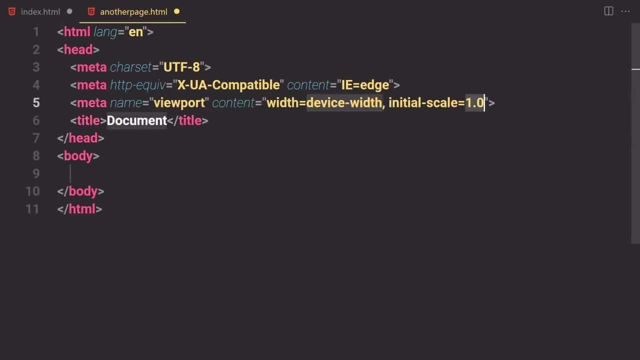 that out anyways. so now let's just write a new anchor tag and it will go to a new file which you're going to be creating. so i'm going to give a name of, like another pagehtml, and now let's just put our doc type in it and i'm going to remove all of this metadata from here and i'm going to 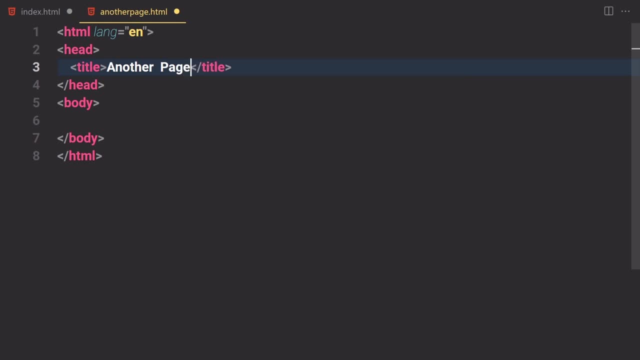 put like another page and now let's just put our content like hello and then paragraph my name is huzzain. and then a new paragraph: welcome to my personal site, and i guess that would be fine. so if you save that, and now let's just link this: 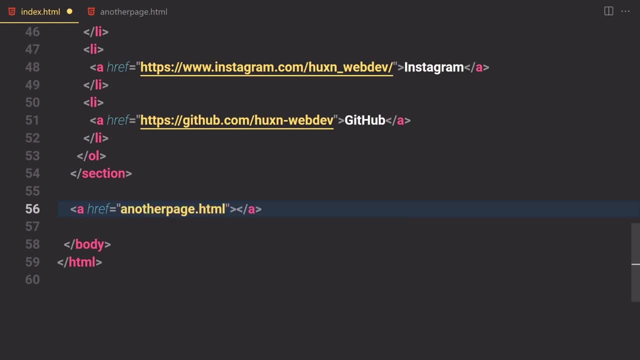 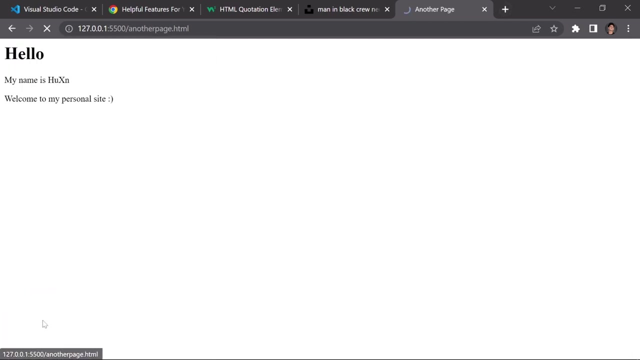 anchor tag to this one. so i'm going to hit ctrl space and then click on another image, another web page. so check out my cool site, ah site to be precise. so if you save that, and now i guess you can see that, yeah, you can see that right there. so if you click on that, so here you. 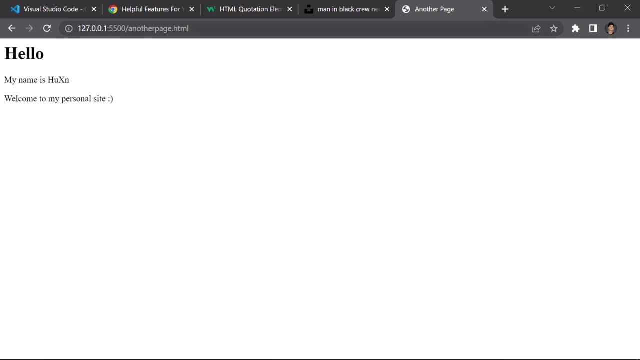 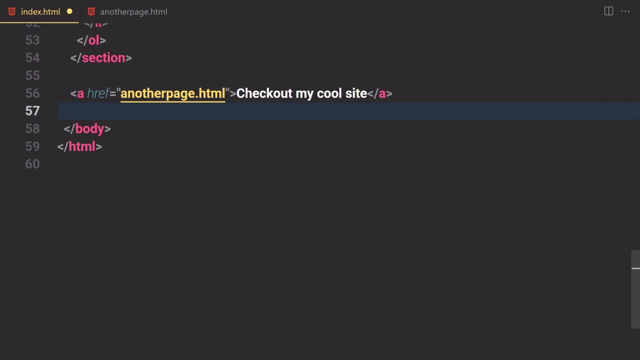 can see what now brings us to this web page: another pagehtml. so we are now getting like: hello, my name is huzzain, welcome to my personal site. okay, so that's that. now let's just write a footer area, or you know what? instead of writing a footer area, i'm going to just create a section. 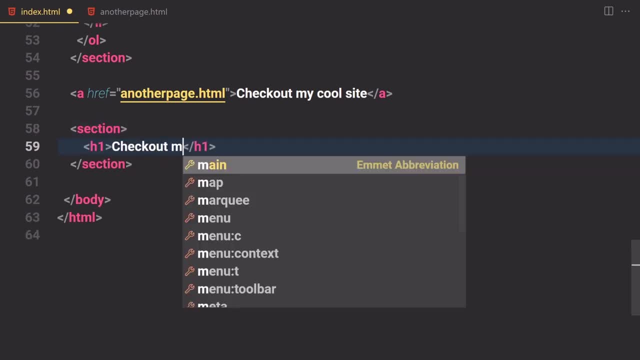 in here and i'm going to write: h1- check out my photography in here and here i'm going to just put and i'm going to give my width of maybe like 200 pixel and also the height of 200 pixel, and i'm going to duplicate this line of code maybe four times and i'm going to have to go. 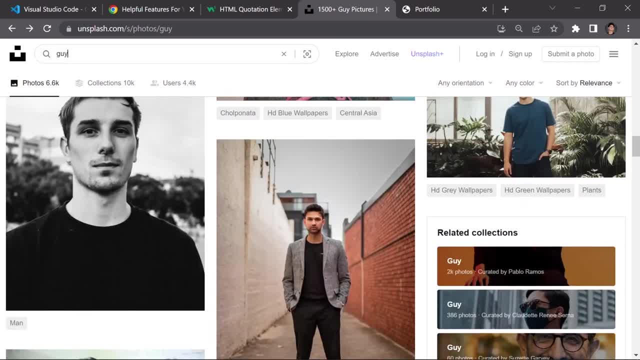 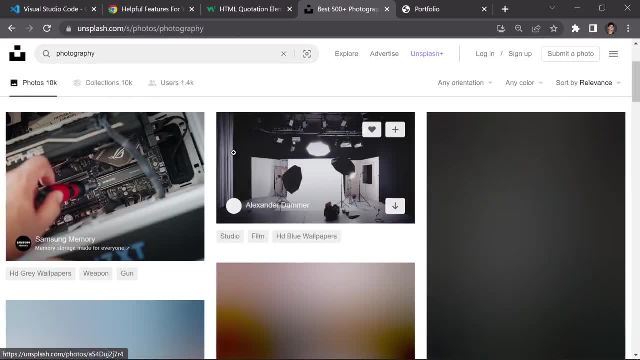 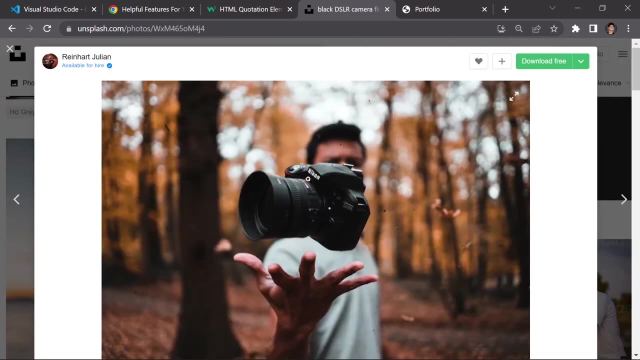 to this unsplashcom and now let's just search for photography. let's just search for photography in here. okay, so we are getting a lot of cool results, but i'm going to right click, i'm going to select that right click on it and copy the image address and i'm going to put this address: 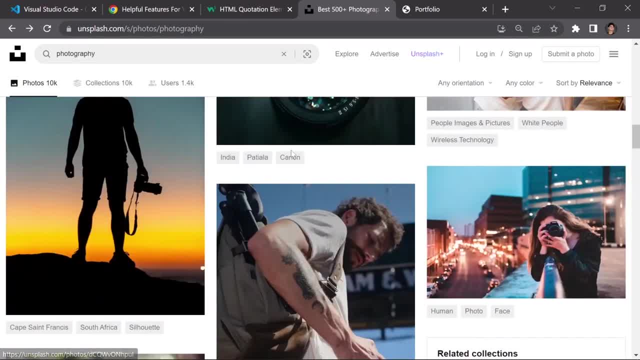 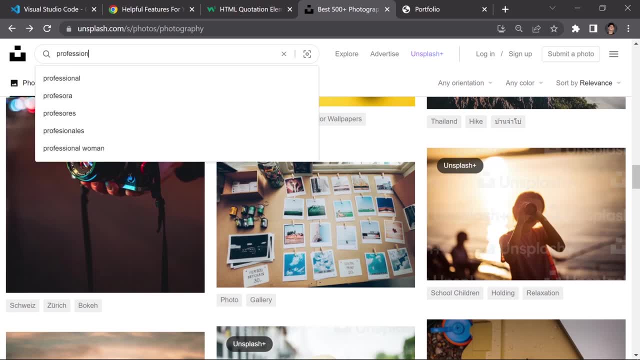 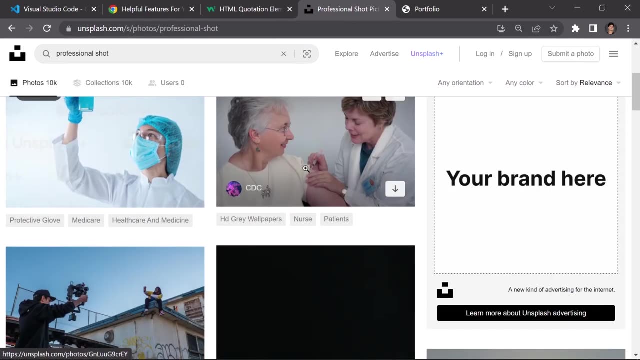 right there. now let's just search for another image. maybe a professional short would be fine. p r o w f, p r o f e double s null uh shot. okay, i can't even speak no more. i speak a lot. professional shot of these people. okay, this is kind of okay. this is a professional shot. right click on it. 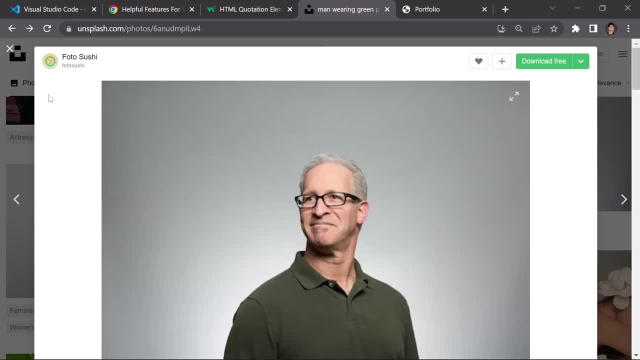 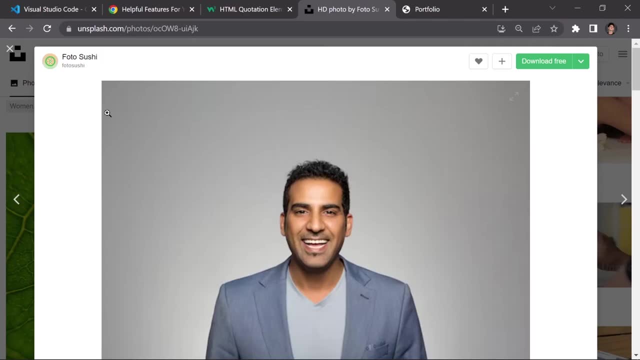 copy the image address. i'm going to put it in here and i'm going to also her image as. okay, this one. all of them are better than the other ones. so i'm going to copy this one and i'm going to also put her image as well. she's also looking gorgeous. i'm going to put her image in here, save it. 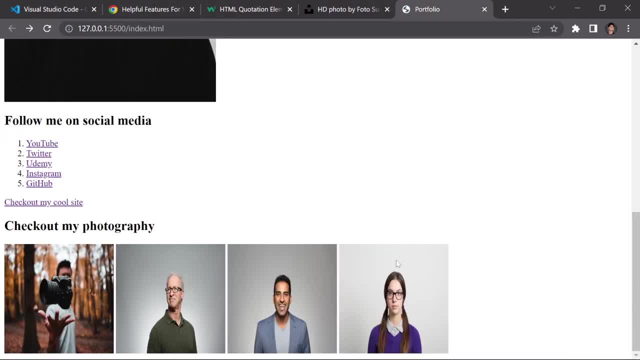 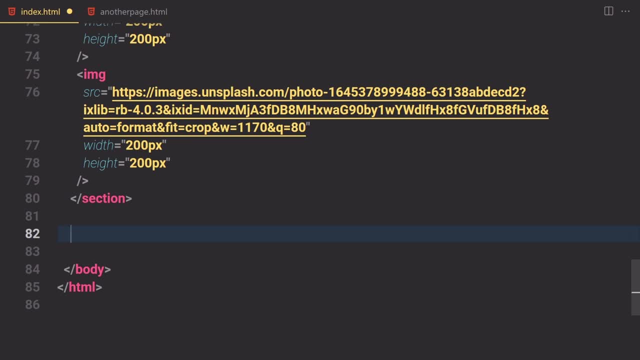 and here my image is like kind of a gallery right here, check out my recent photography and stuff like that. and finally, let's just write our foot section, or we already forgot to include a form so that people can be signed in towards uh project if they want to, so we can just write like input. 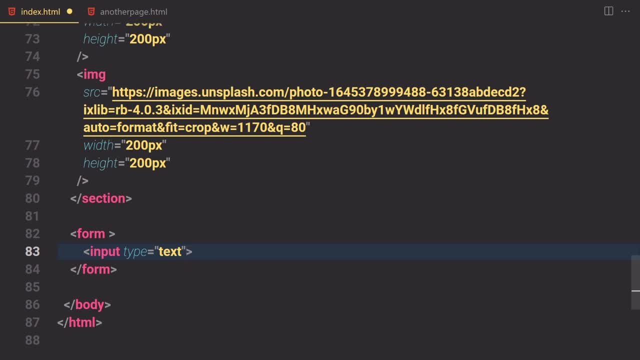 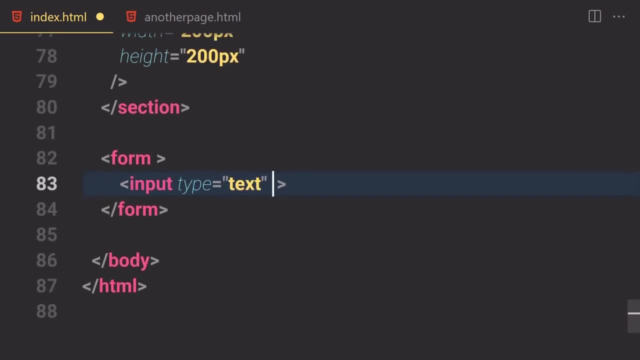 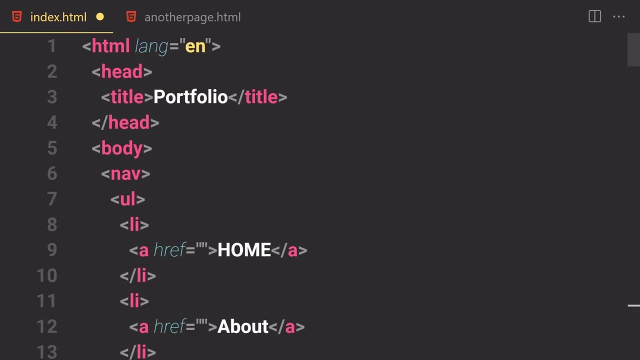 and we can be rude, just like a trader one. and, by the way, i already forgot to include their placeholder in my- uh, what do we call it? a form section? sorry about that. so now let's just learn about placeholders. so you know what i'm going to comment all of these code for now, because 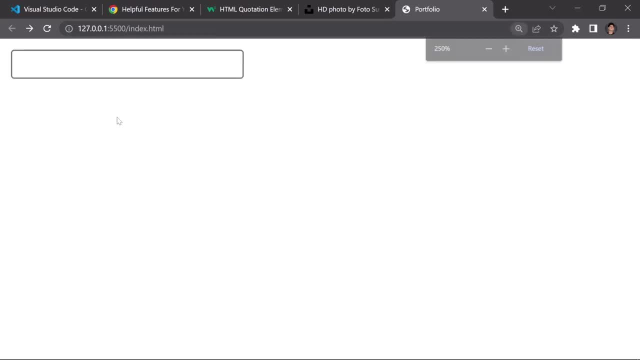 i kind of wanted to show you a placeholder and save it, and now, here you can see, we get a form right here. so in some cases you need a label which will be inside your form, not outside from your form, but inside your form. so if you want a label to be inside your form, so for that we can. 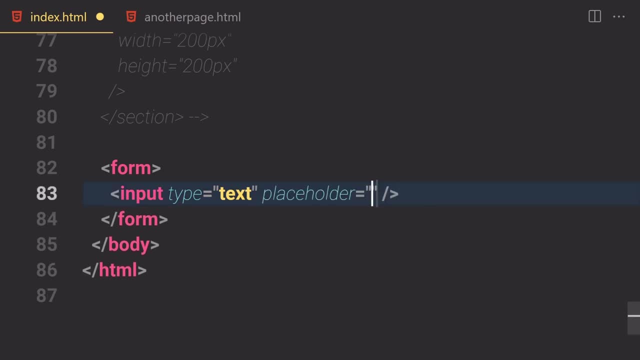 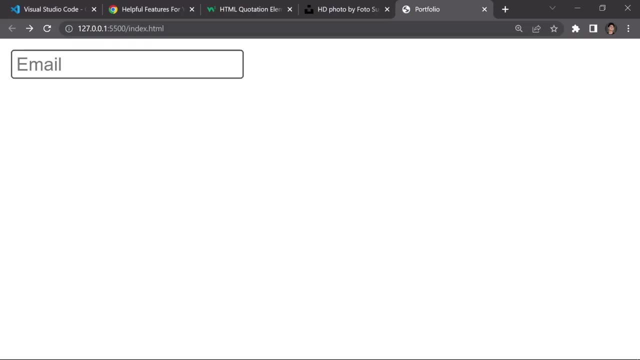 write an attribute called a placeholder and we can write anything we want in it. but here we are going to be just using, like uh, email in here and if you save that and here you can see we are now getting this email right here, and if you start typing something, so that email will be gone. so 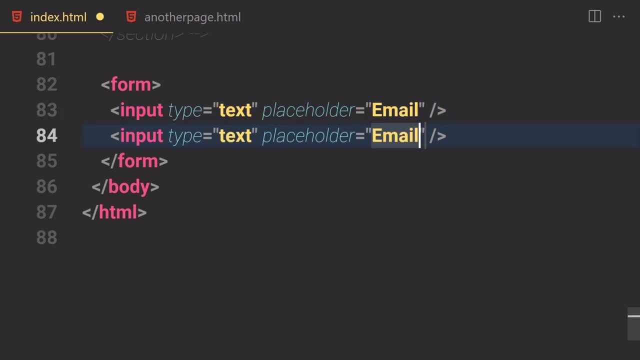 we can just remove that. and here's our email. so now let's just duplicate that and now let's just write our password right here, or you know what? let's just ask for the first name you. so i'm going to write a name. change the text to be like name, not name. but uh, okay, so. 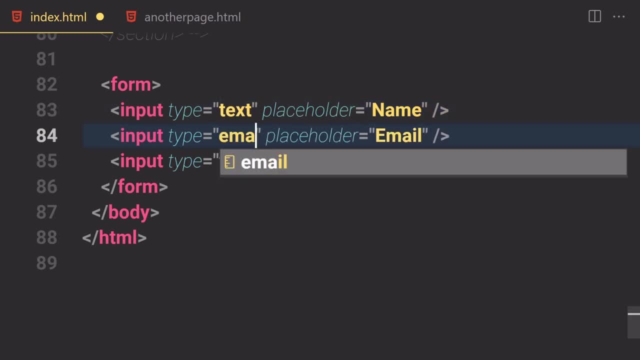 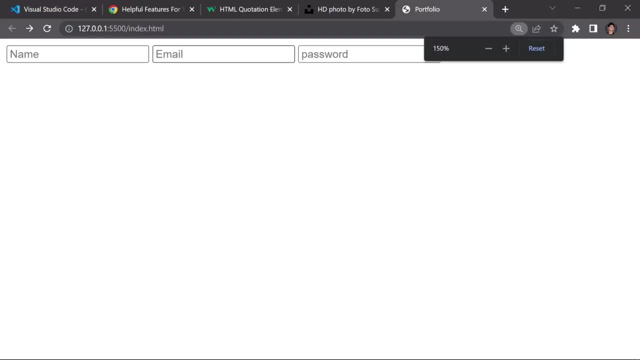 this is going to be the text, and then the next one will be email- kind of lost my mind there- and then here this one will be for password. if you save that, you're now getting email name, email and password and finally let's just write or submit button and we are totally done. 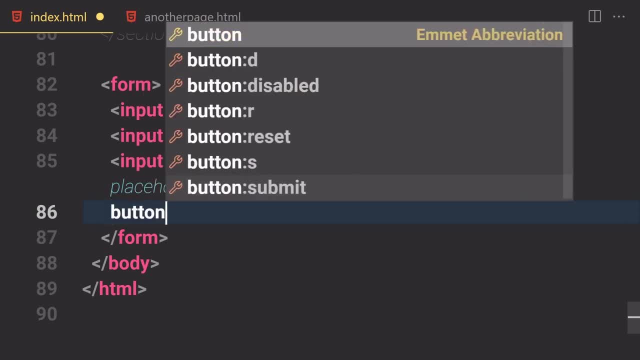 with this project. so, oh my goodness- button and then submit, submit, or you can also create an input, and you can also create an input, and you can also create an input, and you can also create it by writing, and uh, comments. here you can select the option and then select this one comment and 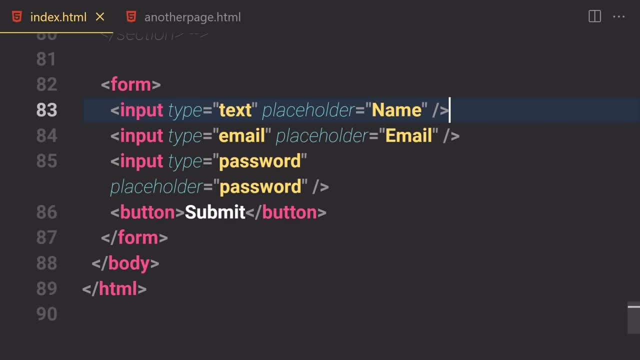 you can wasn't in the issues. and after that we go back into work in the statusеров tool and then we can select the keywords. you get selected- uh, 미안i, in the 71 base and and choose the keyword you Request and we go back into step 1 and we some, we run here, uh, now. now it says: 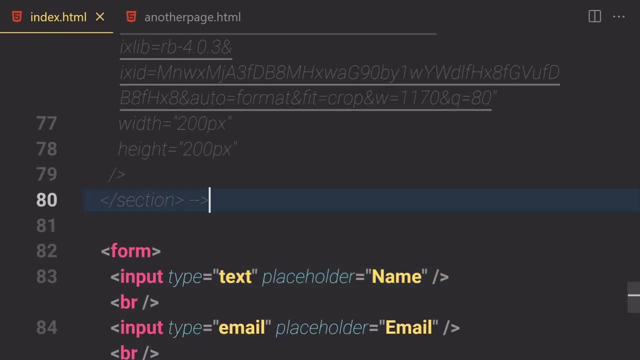 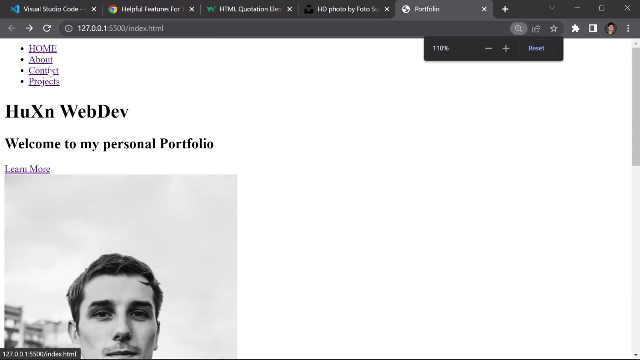 update launcher that you have not done an update, and now it says that, um, you can select a defined using your adapter and then you can decide what you need to update later. so for apples, super command-and- guerrilla, you are going to want to give aluminum buttons so you can repeat. 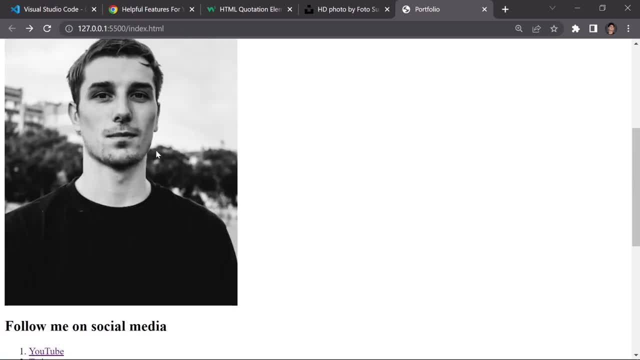 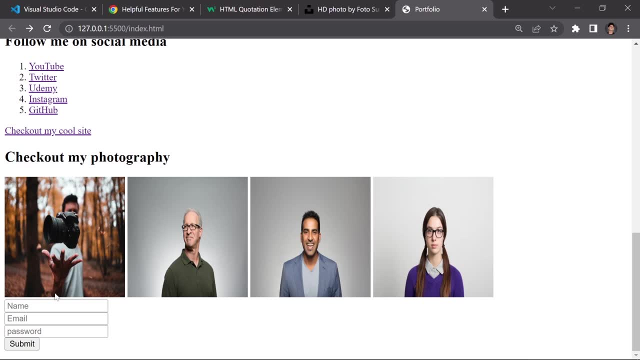 your Ruby instructions if you want to, and here you can see. this is how it looks like. if you want breaks, so we have our gorgeous image right here- look at me. and then we have all of these social media link right here. then we have a photography section and finally we have our 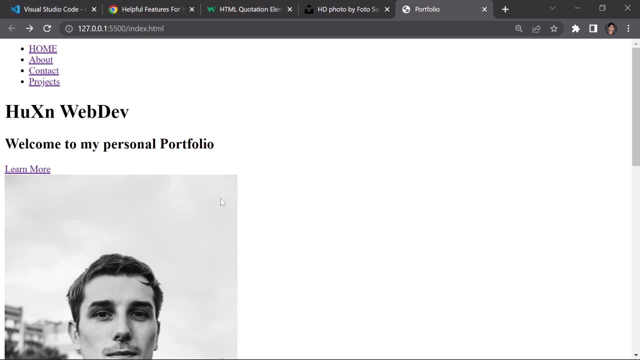 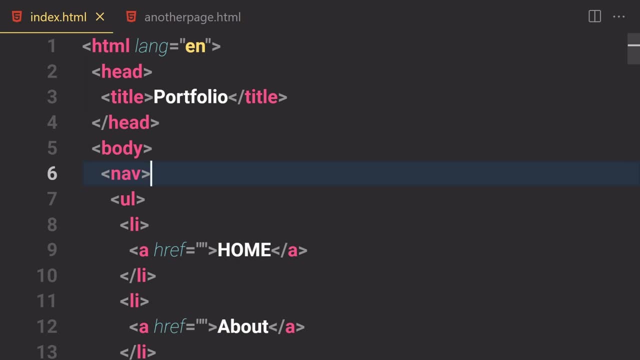 form right here. so now we are totally done with the html side of code. so now the next section. we are going to be learning about crazy amount of css. so by crazy i don't mean like css is hard, css is more simpler and more awesome, and more like how can i put it? like the most easiest. 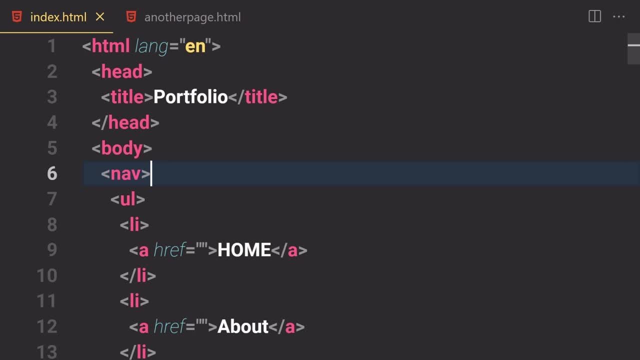 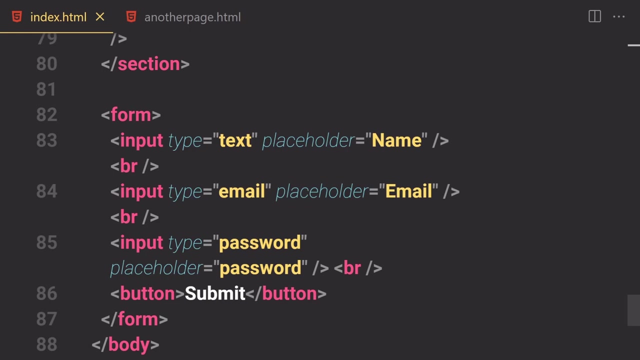 language you can learn. css is easy, but it's a little bit long, so you have to give it a lot of time to learn about css. css is long but it's not hard anyway. so now that we are totally done with our first project and html section, now let's jump into css, and css stand for cascading style sheet. 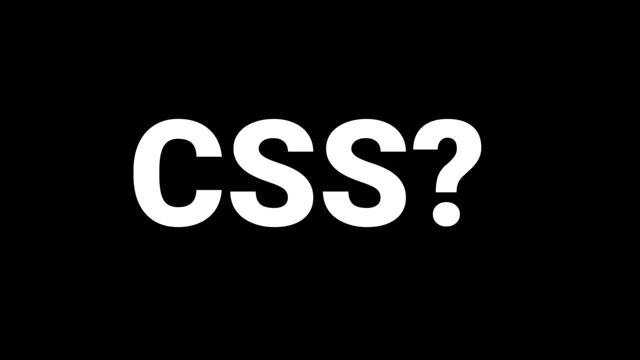 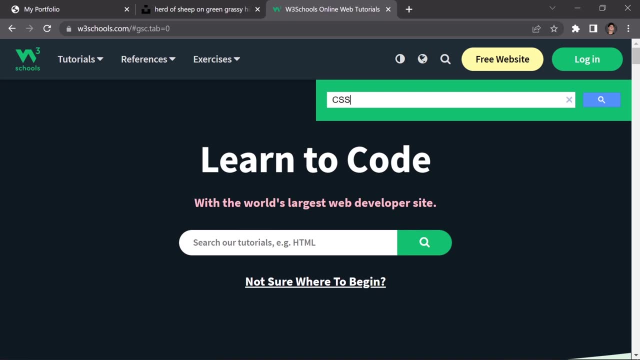 so now let's just ask from our good old friend, like w3 school, and let's just ask him: like, what is a css? css introduction to css. or you can also ask from google if you want to. so i'm going to just click on the first link, like css introduction. 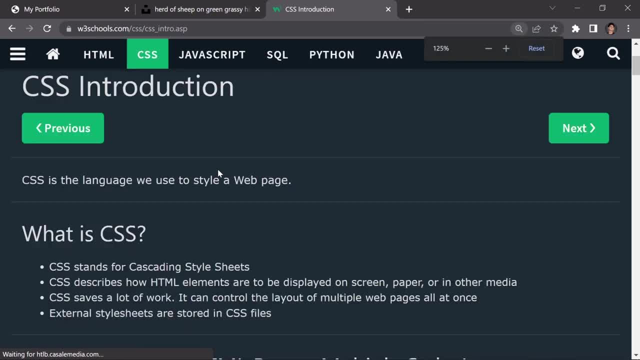 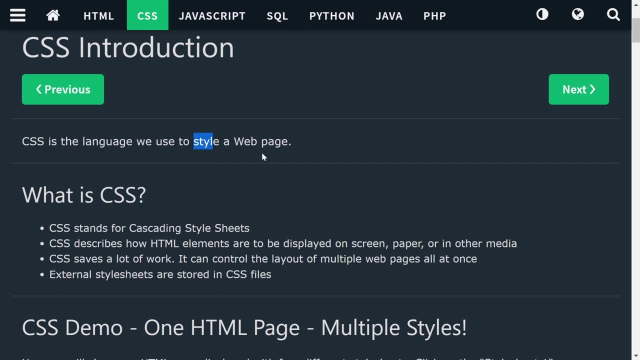 and what is a css? let me just zoom in a bit, like in presentation mode. css is the language we use to style our web pages. a few seconds ago, we just learned about html, and html was responsible for structuring our web pages. and now, in this case, we are learning about a css, and css is now. 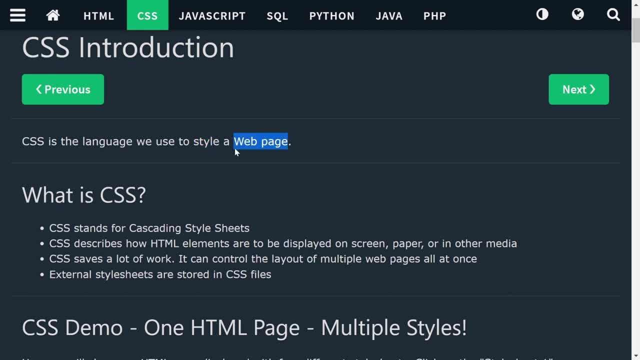 responsible for styling our web pages. okay, so you just have to remember that css is something like a language of a web and it allows us to style our web pages like: this is kind of a marker and colors and stuff you have now which you can use to style your web pages. and so what does even the css mean? 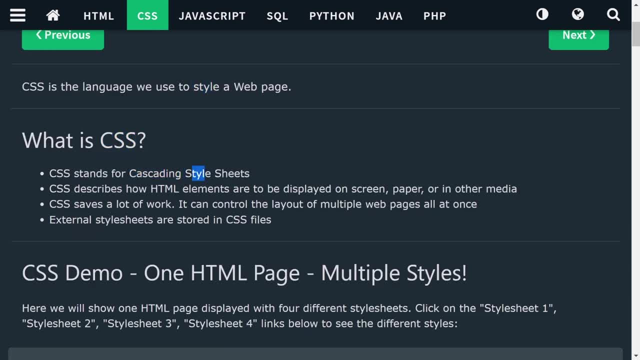 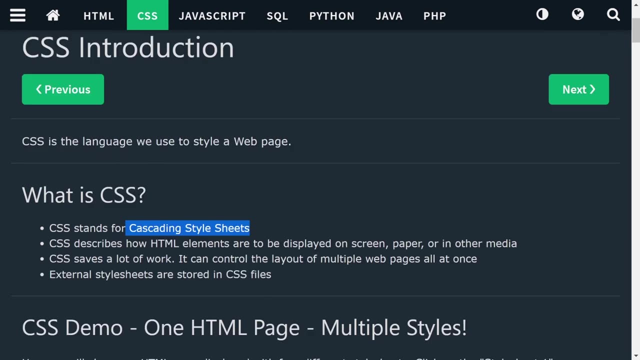 a css stands for like cascading style sheet, so c stands for cascading, s stands for style, and then the other s stands for sheet. okay, so we have cascading style sheet. this is what css means, and then it is a language and which allows us to style our web pages. okay, and css describe how the 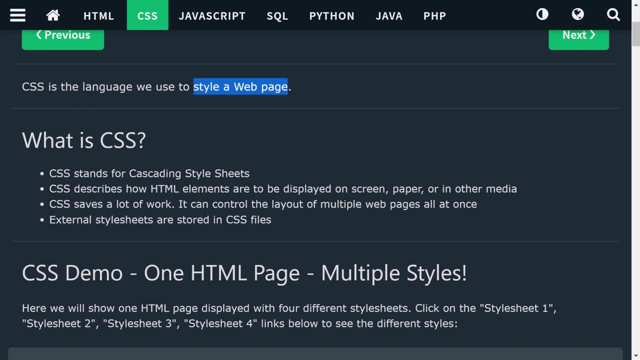 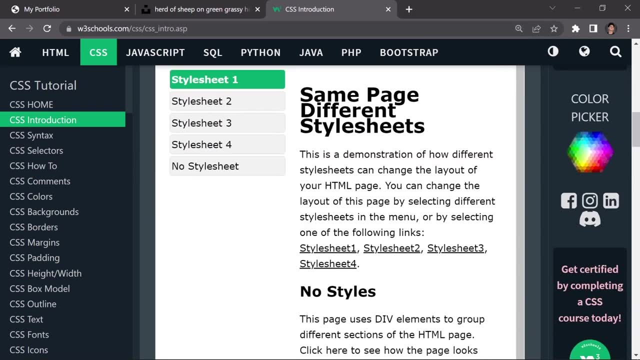 html elements are displayed on the screen paper or in, okay, so you don't have to worry about them from now, which we are going to be exploring in a real great detail, okay, so for now, i want you to just remember these two things, these two lines: like css is the language we use to style our web. 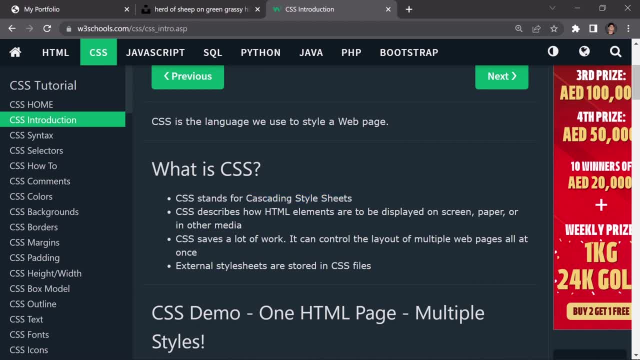 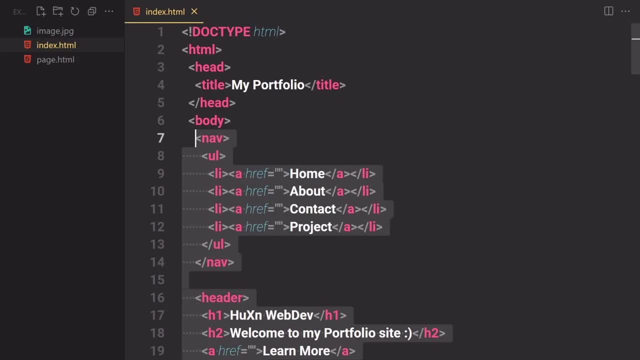 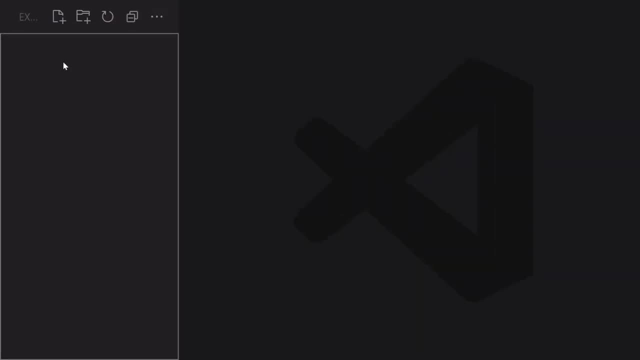 pages, and css stands for cascading style sheet. okay, so now that we know what a css is. so now let's jump into our visual story coder and now let's just start working on it. what i'll do is i'll select everything and i'm going to delete all of them, okay, and i'm going to just zoom in a bit. so 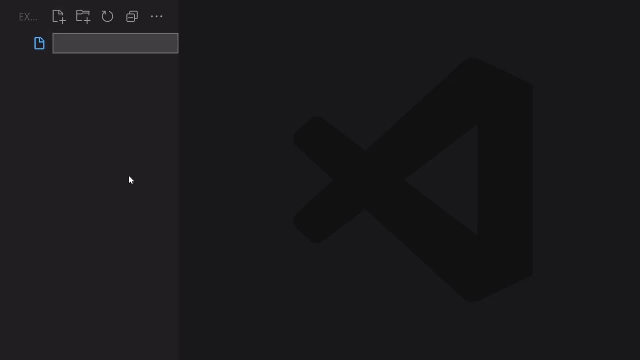 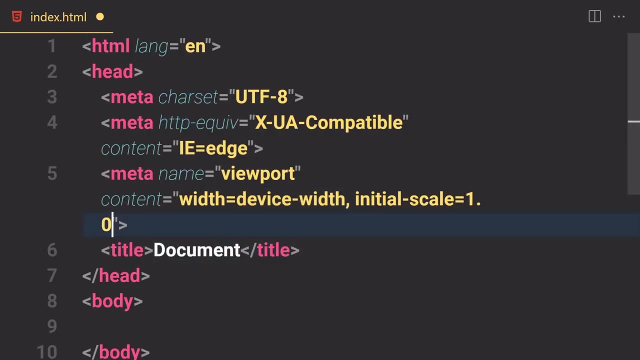 you guys can see everything a bit better. now i'm going to click on this new file and i'm going to just start working on indexhtml from scratch. okay, and here i'm going to just write a doc type html thing from scratch. one more time, and here inside this section, we are going to be learning about css. 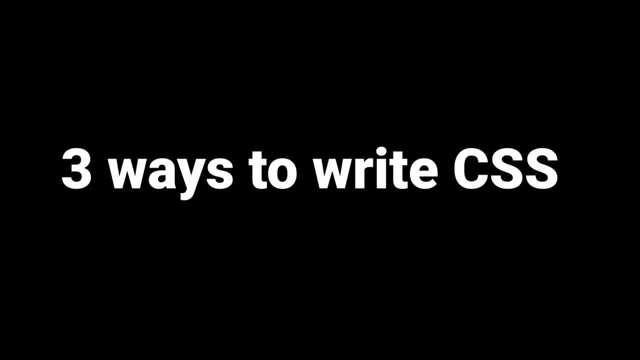 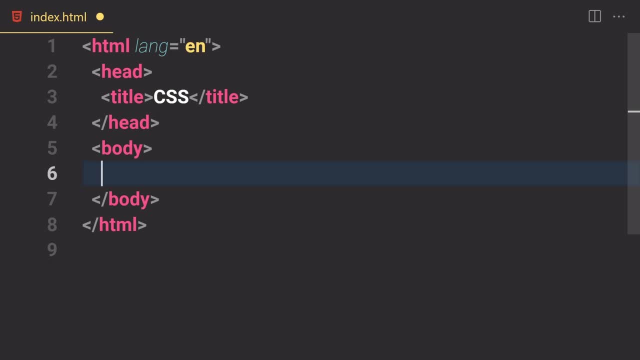 so i'm going to name it as css. okay, so now that we know what a css is. so now let's learn how we can connect our css with our html. okay, so there are three ways we can connect uh css with html. so the first way we have is an inline uh css, or you know what? i'm gonna write that in uh heading. so i'm 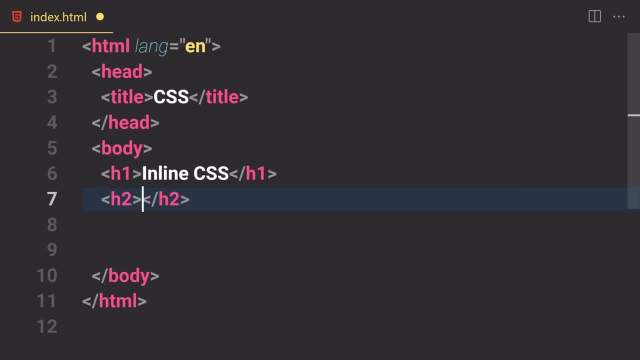 gonna write h1 of inline css, and then i'm going to write h1 of html, and then i'm going to write inline css, then we have, uh, internal css and then finally we have our external csn, and i love external css. okay, so if you save that and if you go to our browser, it's complaining, so right click. 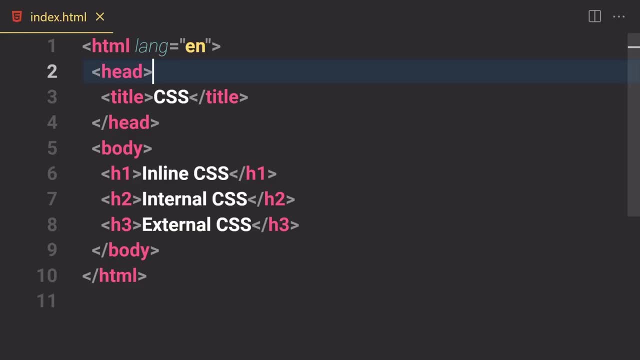 on it and open it with the live server, and now we are good to go. so how can we apply a css to just inline text, like, maybe i just want to provide a styling for this one h1, or maybe for h2, or or for h3, or even for a body? i can also provide styling for a body if i want to, and we are going. 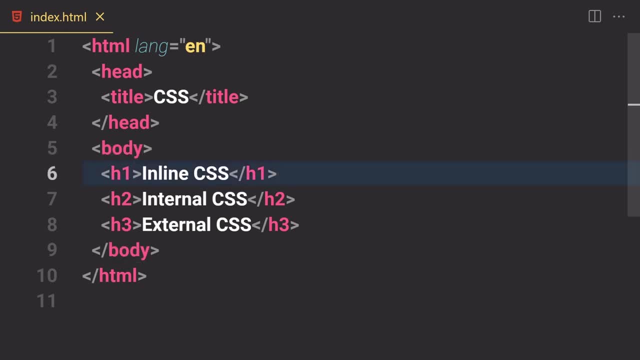 to be learning about crazy css in this video. but if you want to apply css to just one element, so we can either use inline css or ex internal css or external css. okay, so suppose if you want to work with the inline css, so for that we just have to first of all select the element it doesn't. 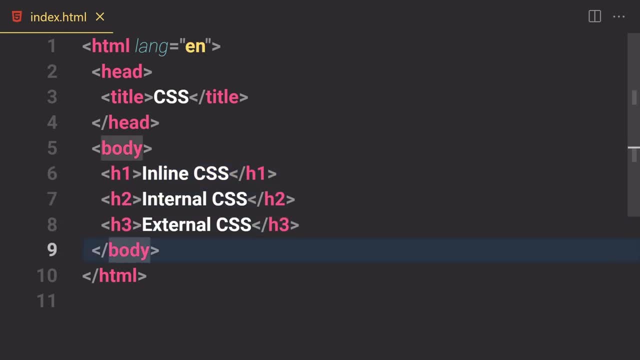 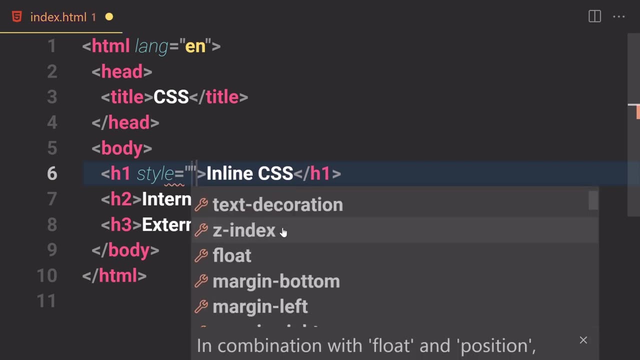 matter if you want to select this one, this one or that one, or even a body or whatever. okay, so we here just a style attribute, and here you can see all of the css properties and its values. i'm going to tell you, like, uh, how the syntax of the css looks like, but before i do, i just kind of want to. 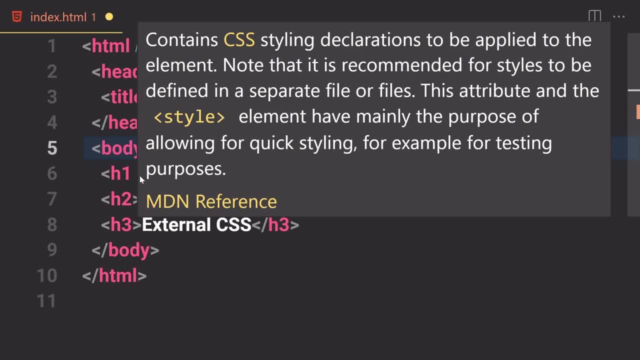 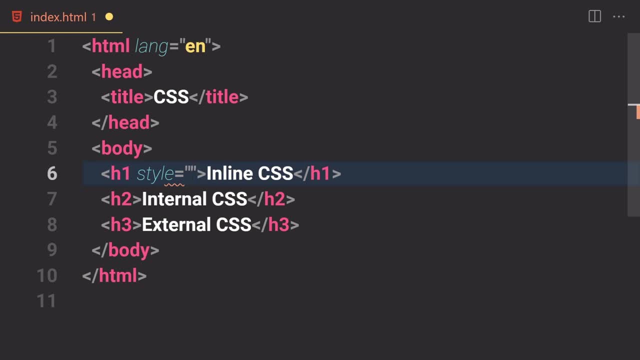 tell you like how we can write an inline css. so first of all you just have to write a style attribute and then here you just have to write our property and its values, and i want to tell you like what a property and the value is in a second. but you just have to write like color, and then 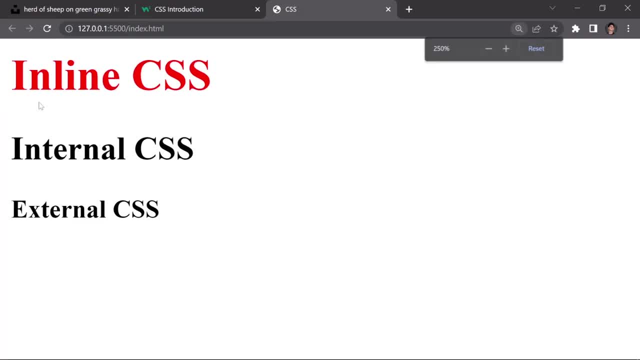 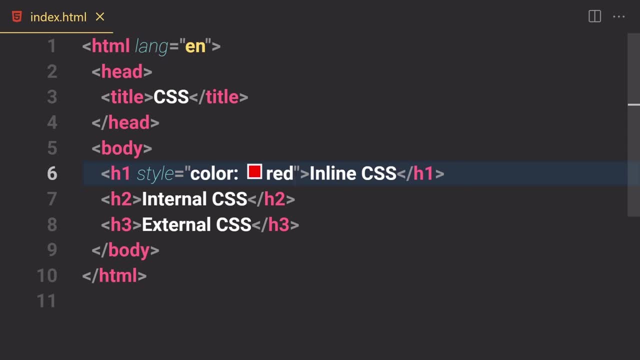 like red, okay. so now, if you save our file and boom, this is our first inline css, right here and now we just change the color to be totally red, right here, okay. so this is known as an inline style and we are not going to be using inline style ever. i shouldn't have to say ever. we will use in some cases, but these are not. 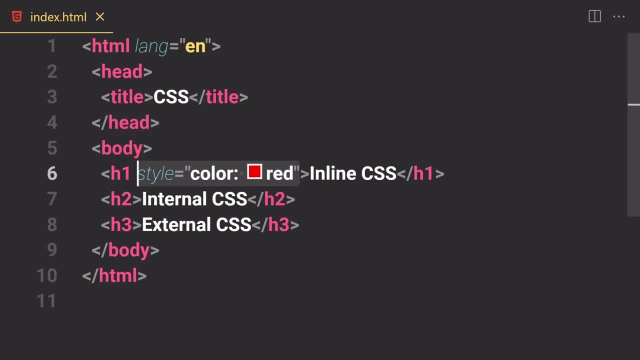 useful because we have to, like uh, provide uh starting to each of the element we have to select there. like uh. we have to copy this style attribute and it will look messy, like let's suppose we change it. so let me just give you this example: if i pass it right here, pass right here. and if i 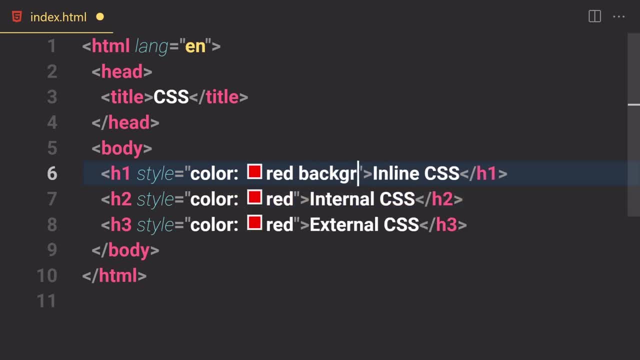 type uh like something. you don't have to type everything which i'm writing, but i just kind of want to give you an example. like background color will be like uh, crimson maybe for some case, and if i just started typing like so, so my code will look messy. so we are not going to be writing. 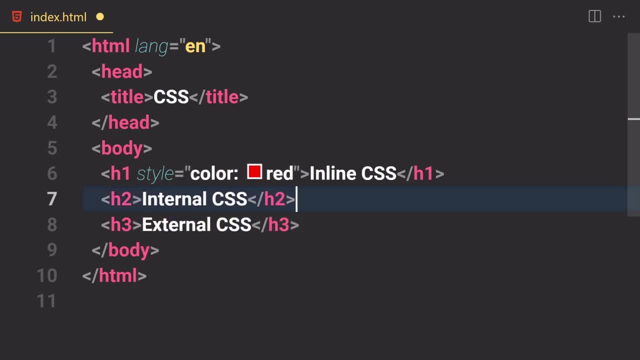 or inline css, maybe ever, but i shouldn't say ever, because we will just need it for some cases. so now, if you save file and you already know that, call this change to red. that was it about inline css. now, then the next one we have is internal css. internal css will be. 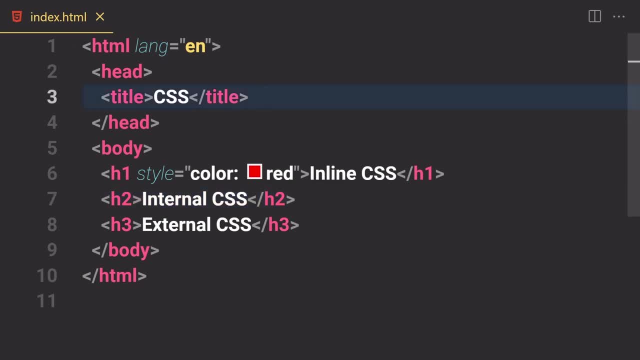 inside or indexhtml file. okay, so we just have to write inside the head area. we just have to write like style, and if you hit tab, so run along, gives a style opening tag and style closing tag. and now, inside this style, we first of all have to learn about the syntax of css. so now i'm going to just 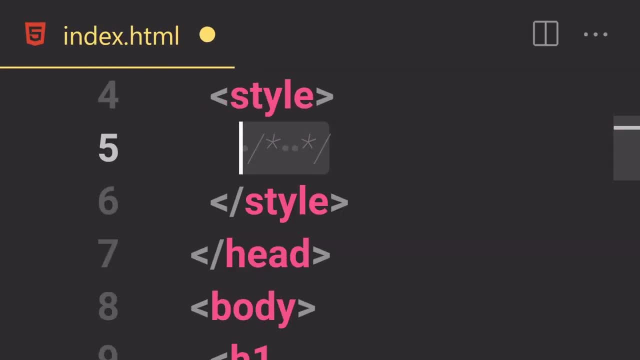 zoom in a bit so you guys can see everything a bit better. i want you to just focus on this area right here. so how the syntax of the css will look like. well, first of all we have a selector. okay, zoom out a bit, a little bit. so we have first of all the selector, then we have opening, curly brace and 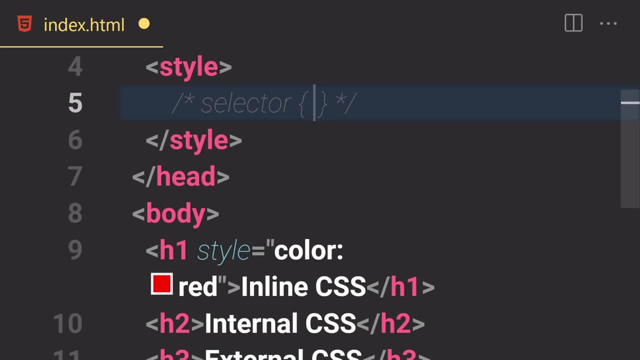 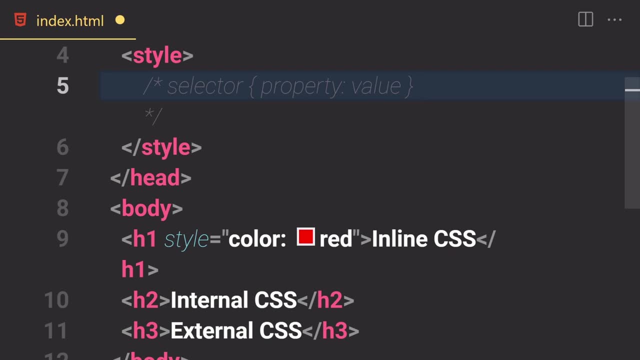 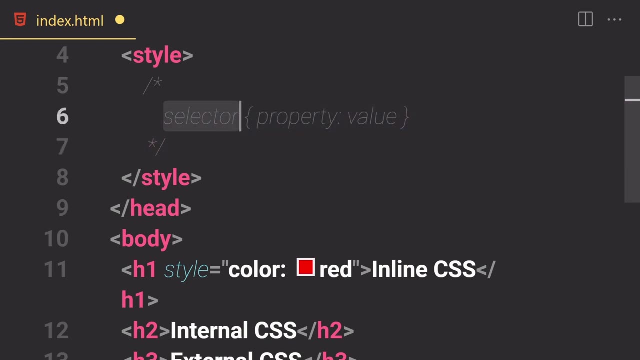 then the closing curly brace, okay, and now inside that we are going to be writing a property and then value of their property, okay, so this is just a css, uh, syntax first of all. uh, let me just hit enter right here. first of all, we have a selector, like some sort of a selector, and we 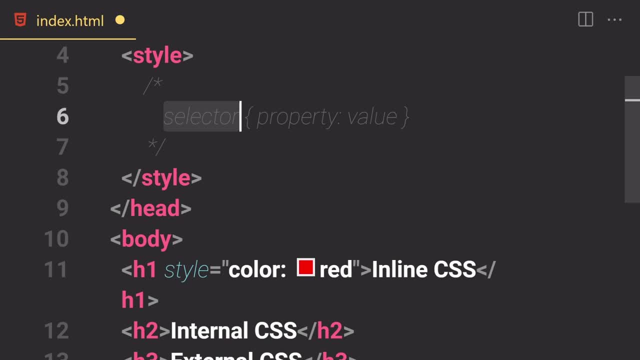 are going to be diving into our selectors in a real great detail, but you don't have to worry about them for now. users have to remember, like, if you want to work with a css, first of all we have to write some sort of a selector. we want to select something like: we want to select h1, h2, h3, header footer. 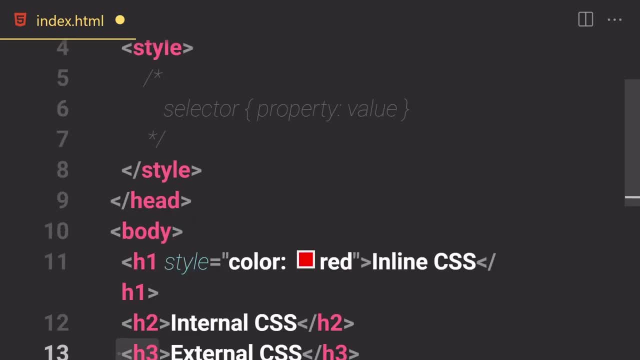 section navigation: uh, alternative text or alt or image or anything. we need to first of all select that element, then we have to write a opening curly brace and then the closing curly brace. then we are going to be using a property and then specific value of that property. like, let's suppose, if you want to write a color, 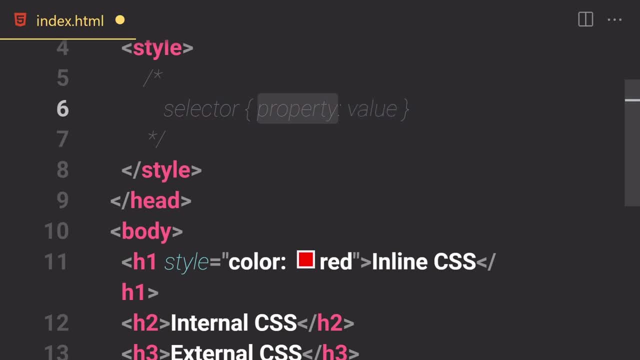 so you have to provide a value of the color. you want to change the background color? you have to provide a background color value. you want to work with a display property. you are going to be using a display value right here. so this is how the css syntax looks like. 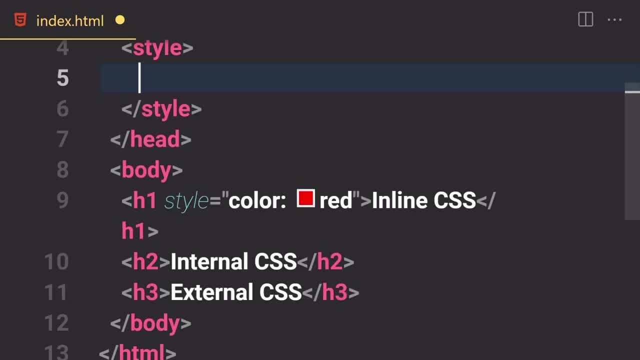 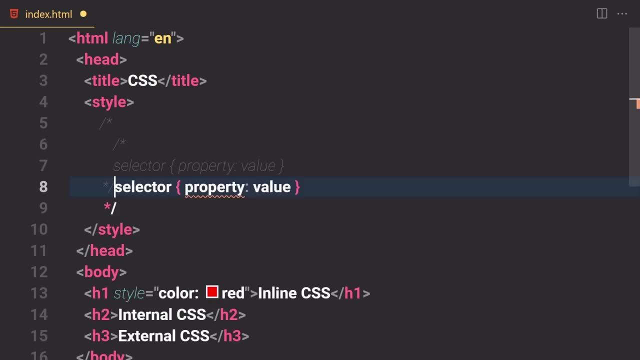 and now we are going to be diving into it. so i'm going to just cut that from here, and now let's just zoom out of it, and now let's just pass it in here one more time. so, oh, my goodness, i'm just passing in again and again, all right. so now, if you want to select something like in this: 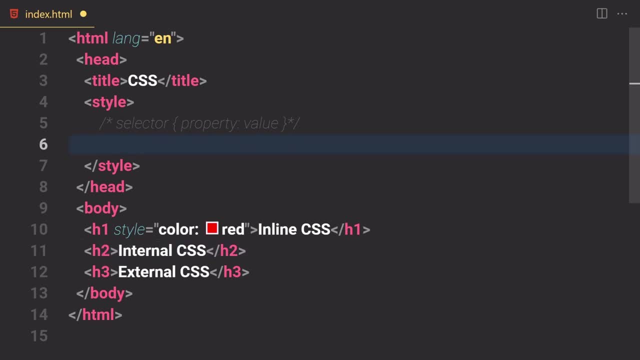 case, if i want to select h2. so what do i have to do? i'm going to just write h2. so now the first step is complete, like the selector step is complete, like we selected this h2 successfully. now what else do we have to do? we have to first of all write opening, curly brace and then closing. 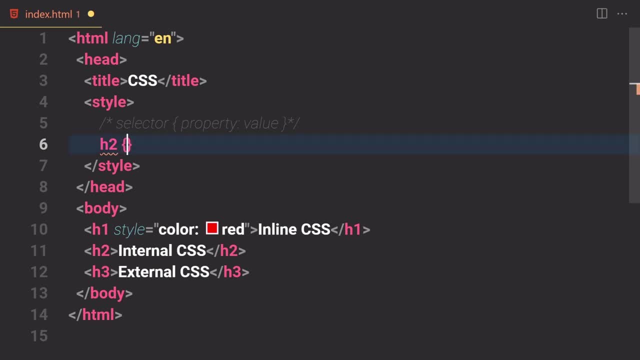 curly brace. so i'm going to just write opening current libraries and then closing curly brace, and now inside there we are going to be using a property and its value. so which kind of property we have? we have, like countless properties in css, but for this specific one we are going to be just 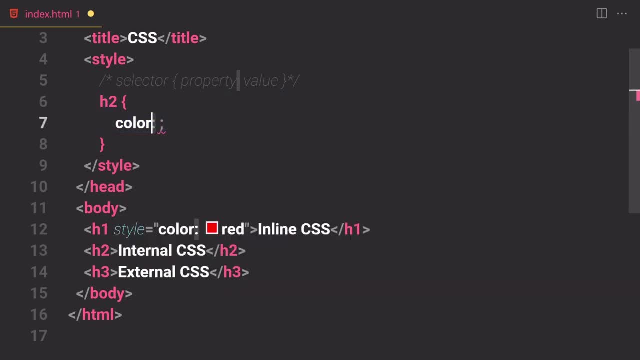 using like color and if you hit tab so it will not give us like this colon and this semicolon right here. so here we are going to have to provide some different color. so if you hit control space, it will give us a lot of colors right here. i can't even pronounce the name of these colors right here. 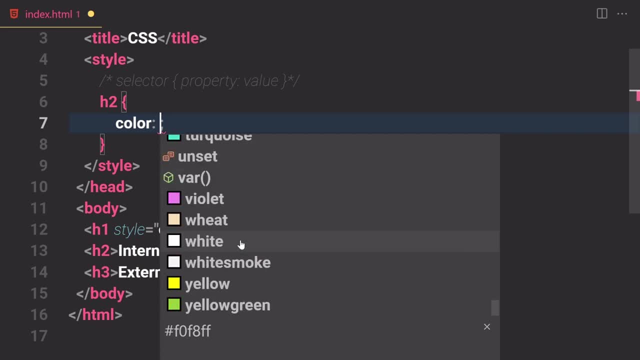 like. there are a lot, a lot of colors here you can choose from. so i'm going to just click on random color like uh, i mean like just doji blue would be fine, or you can just go with the blue if you want to. so if i save my file and boom, here you can see this will now first of all select this. 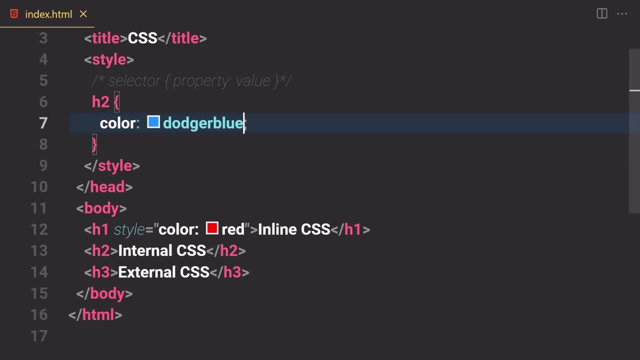 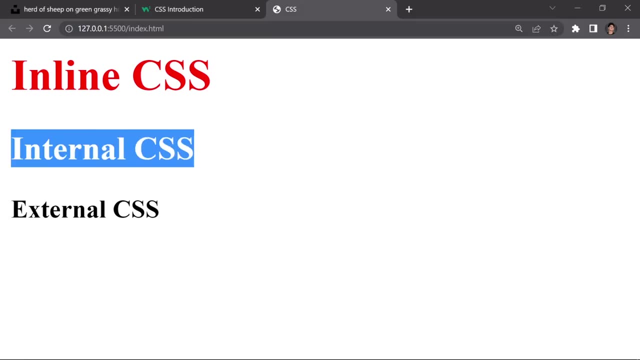 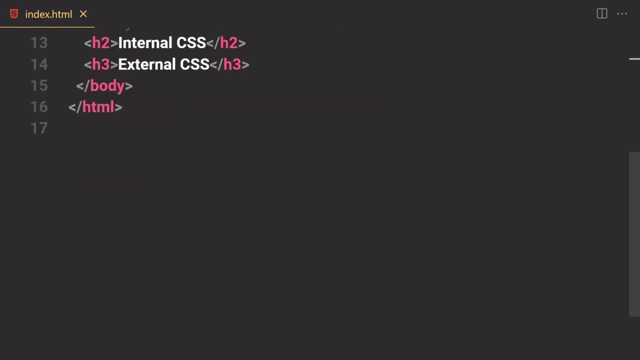 element and it will now provide this color to it right here. okay, so we can also provide just a blue color if you want to. so if you save our file, so what do we get? we get a pure blue color right here, but this is also not the best way to write a css, because we are going to be writing a lot like a 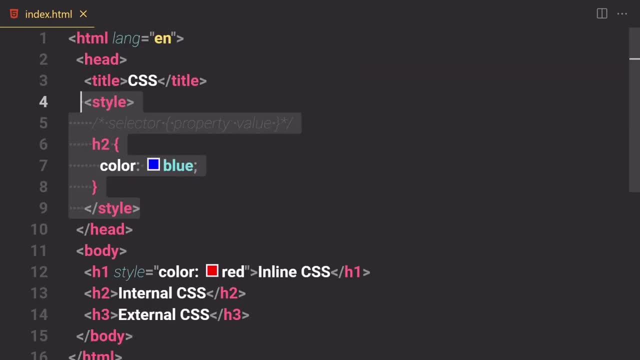 lot of colors right here, so we are going to be writing a lot of colors right here, so we are going to be writing a lot of uh html code. but if you write a html and css code at one file, so our file will look messy and no other developer can work with that. so this one method is also failed. but 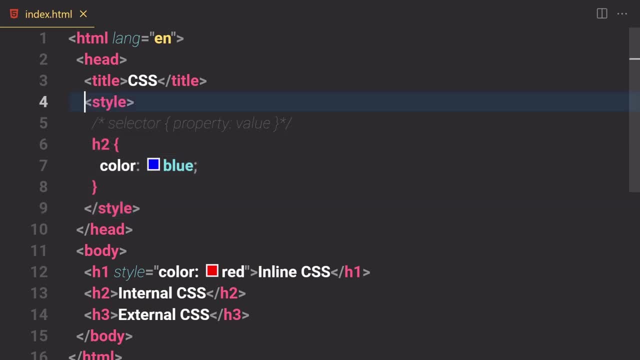 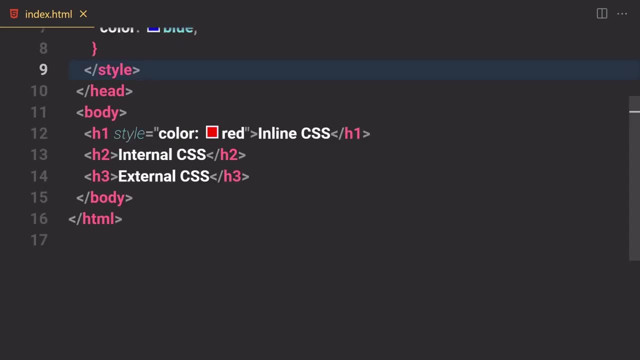 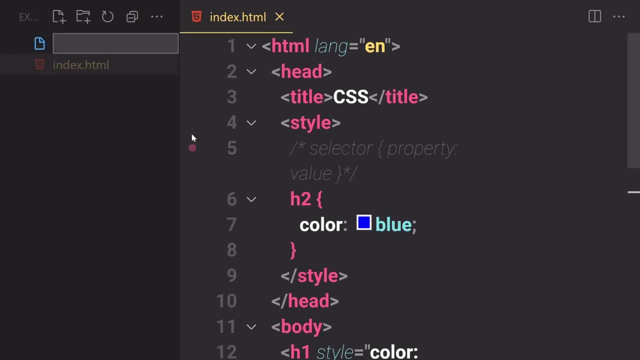 you will, in some point in your life, use this internal css as well. and now let me show you the last and the final way, and my favorite one, which is known as external css. so now, first of all, we have to create a new file for that. so i'm going to just write like: uh, let me just zoom in a. 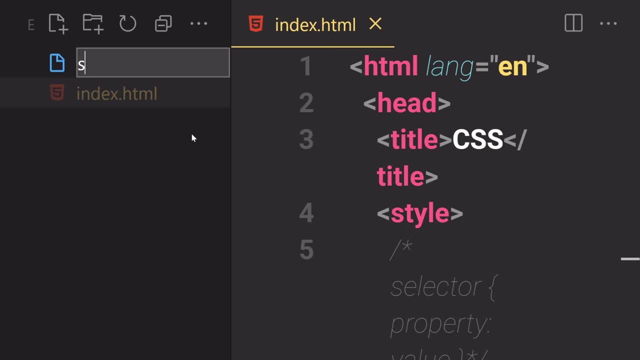 bit so you guys can see everything a bit better. so first of all, you just have to write some sort of a name. but remember, css extension is important. you have to give this like css extension right here and now. you know like what is a css? a css is just a language for styling or web pages. 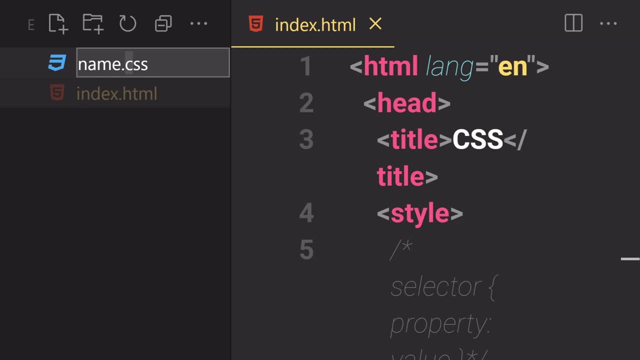 and css stands for, like cascading style sheet. okay, so first of all, you have to write some sort of a name. it doesn't matter whatever name you provide, but you don't have to give my spaces in here, okay, so let me just write a name and then i'm going to give it a name, and then i'm going to. 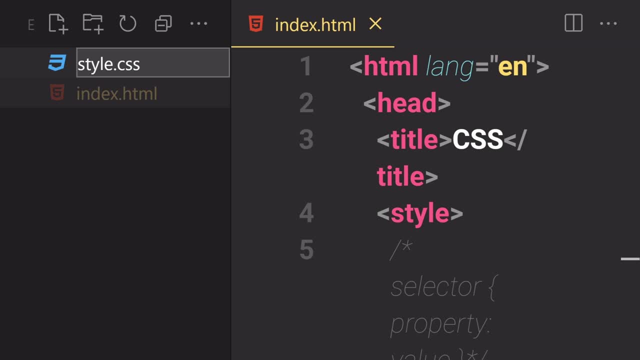 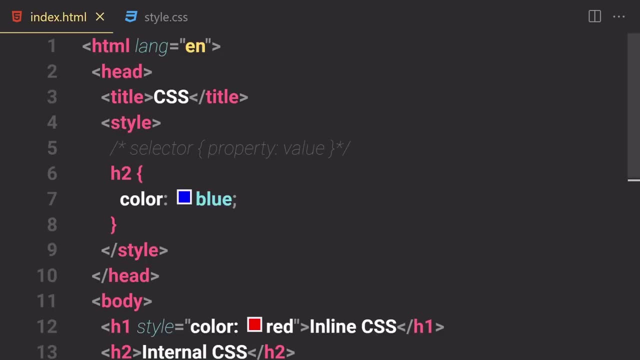 give it a name of like: uh, i don't know. i'm going to write like stylecss would be fine, so i'm going to hit enter right now. so now we successfully create our css file right here. so what was the syntax of css? i'm going to cut this syntax from here. i'm going to paste it right here, so we have. 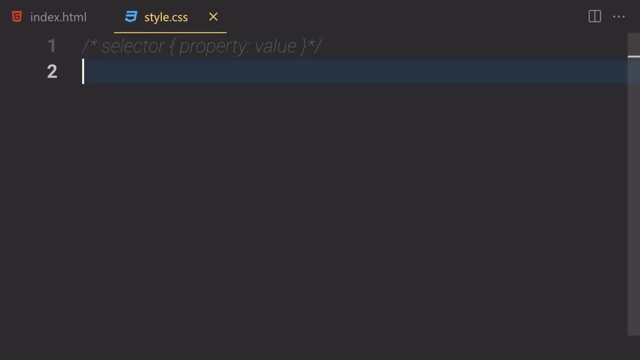 first of all selector, then the opening curly brace, then the closing curly brace, right here, then the property and its value. okay, so i know i'm repeating myself, so i want you to just uh remember this stuff, so that's why i'm repeating myself. so now, in this case, if you 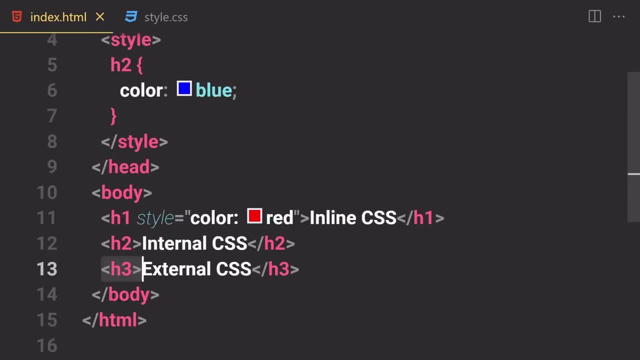 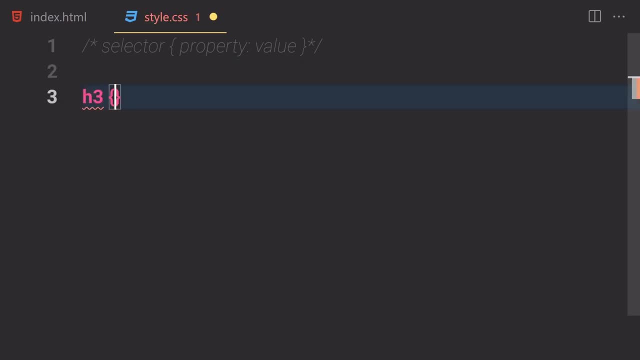 want to select this h3. so what should i do? okay, so i'm going to just head back over to my css file and i'm going to just write h3. so now the first step is complete. then i'm going to write like opening curly brace and closing curly brace. okay, so the second step is also complete, and then i'm 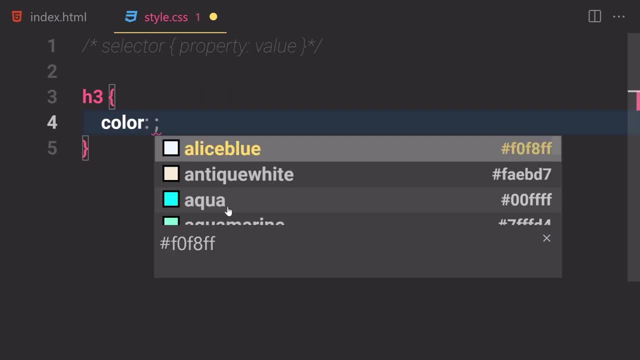 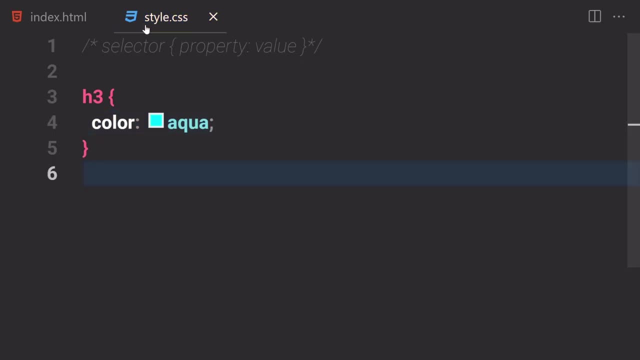 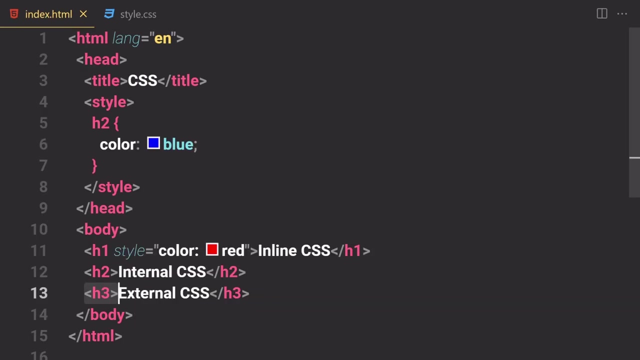 going to write a property name, color, and then this value will be like: aqua would be fine and knife is. and now i want you to just notice: nothing happened. why? because we do create our css file, but we didn't connect that with our html file. so now, if you want to connect this css file with our html file, so what? 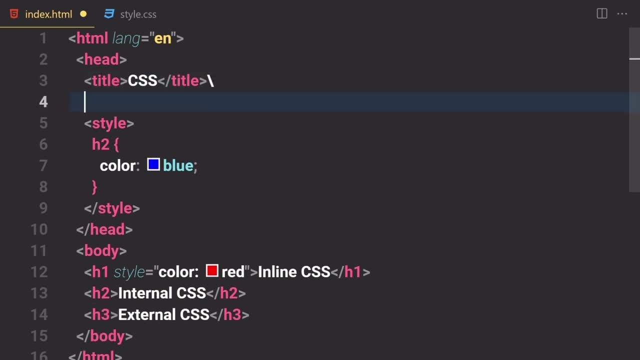 do we have to do for that? so, underneath this title, what do we have to do? we just have to write a link. if you just write a link and if you hit tab certain log uses two attributes. so the first attribute we have is a link, i mean like a rel, and it will be now set to like a style sheet because we are working. 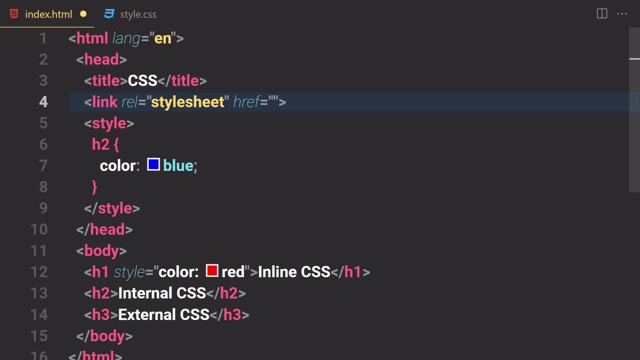 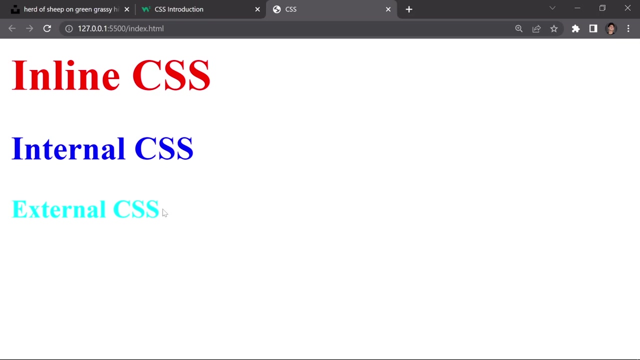 on a style sheet and then here we have to provide the url of our specific style sheet. so we have the description here. so if i have a sql file that is different from the one i had, people, you can see in the description what i'm going to do. i'm going to hit ctrl and space and then i'm going to select. 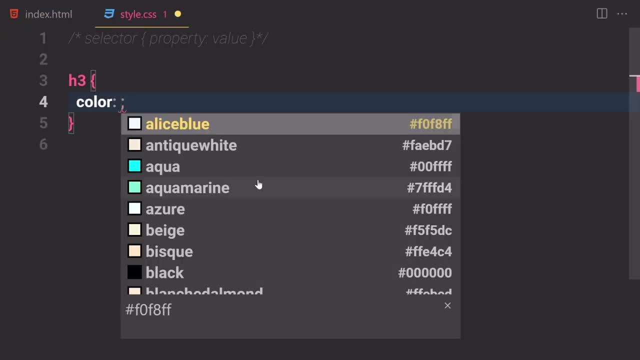 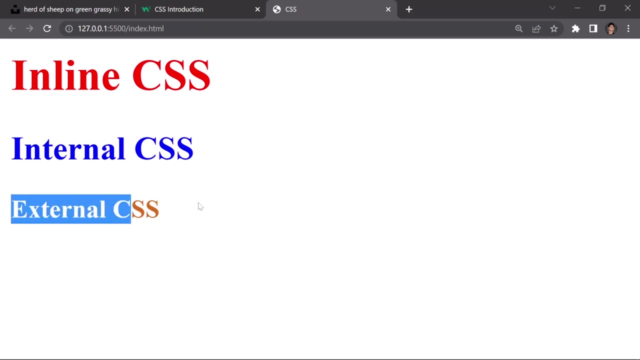 my stylecss file and knife is out there and boom, look at this aqua color right here. okay, so let me just change that to like some other colors that you guys can see everything about better. maybe coral will be fine. no, i'm going to go with the chocolate. i'm going to save my file and here you. 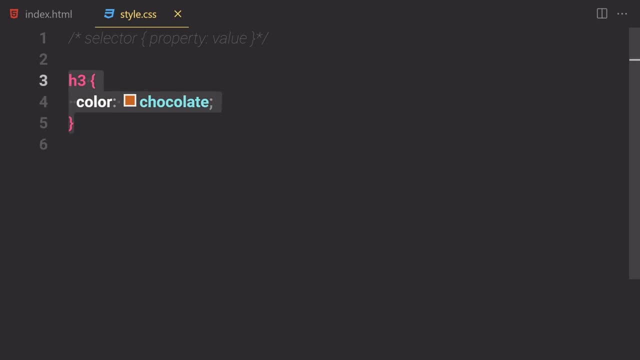 can see we get a chocolate color right here. okay, so this is the better and preferred way to use a css throughout this course. what i want you to do is that i want you to delete the stylecss, or just a style, from there, and i also want you to remove all of this stuff from here. so i'm 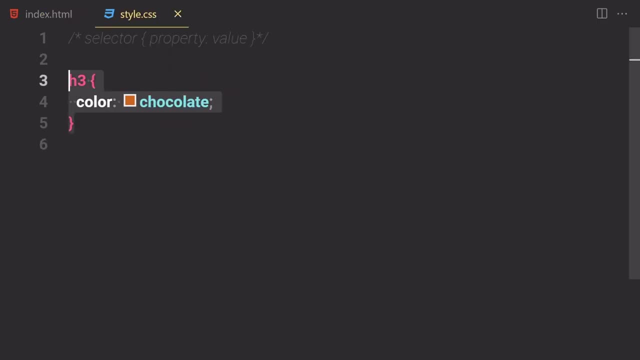 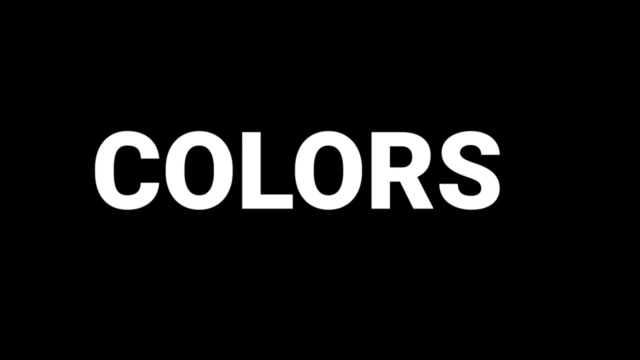 going to remove that, and if you save that, everything is gone. okay, so i'm going to also remove this h3 from there. so now we have a clear file right here. so now that we know how to work with the css. so now the next thing which i want to tell you about. 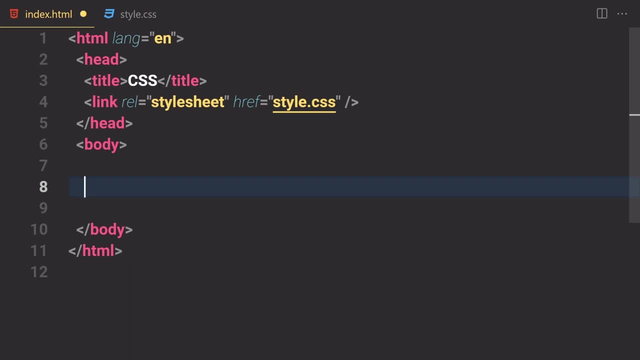 a css. is that how we can work with the colors by using a css? so first of all, i'm going to write h1. so the first way we can work with the css is by using color names. and now, the second way we can work with the css is something called rgb, and we are going to be also learning about rgba. and now, 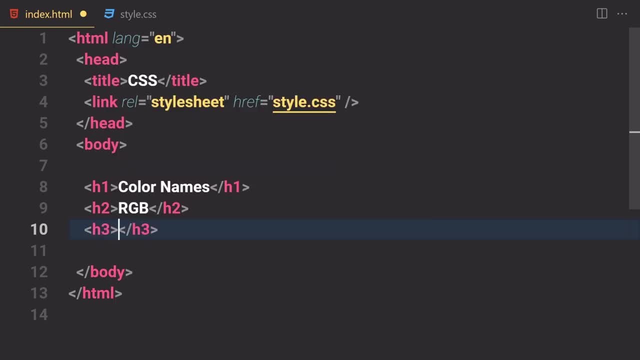 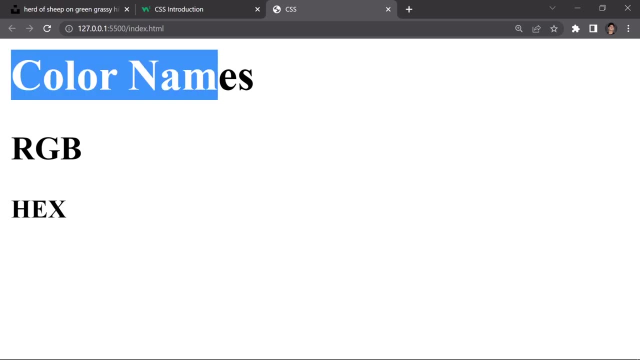 the third way we can work with that h, i mean, like css is called hexadecimal, so i'm going to just write hex in here and now, if we save that and we just get, like, uh, color names, and then we're going to be able to work with the color names, and then we're going to be able to. 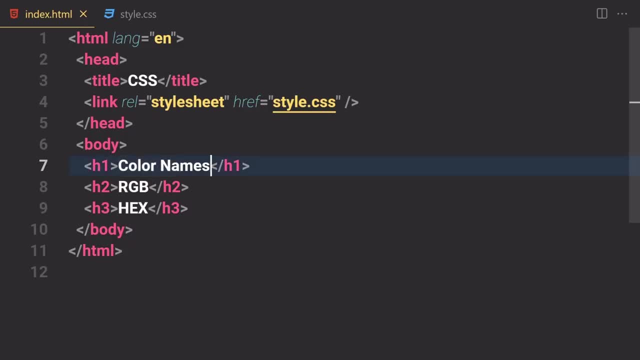 rgb and then hexadecimal color color name. so if you want to provide a color to this specific element. so first of all, what do we have to do? we have to first of all write h1, like we have to select that. then we have our opening and closing curly braces and then we have to write color. 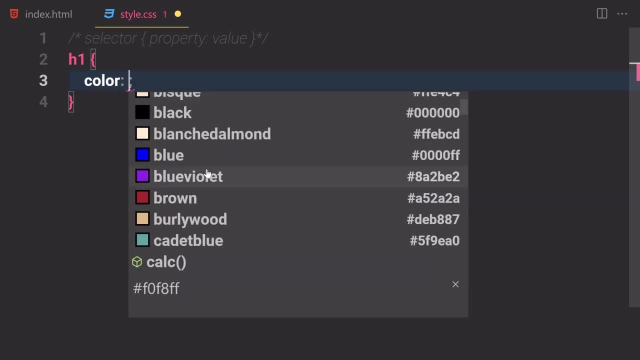 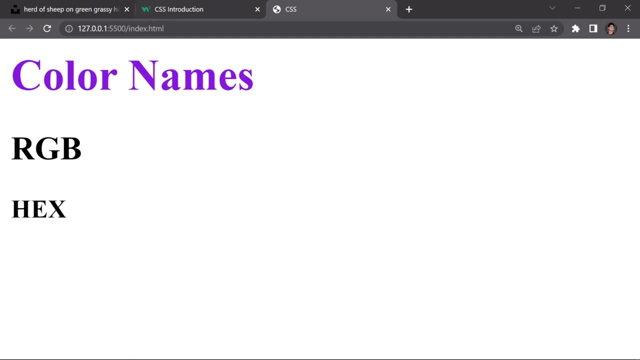 property and then the value to that color. like you can choose different kind of colors from here, like in my case, if i want to choose this blue violet color, so i'm going to click on that and now, if we save that, and now here you can see- it will now change the color to like blue violet. 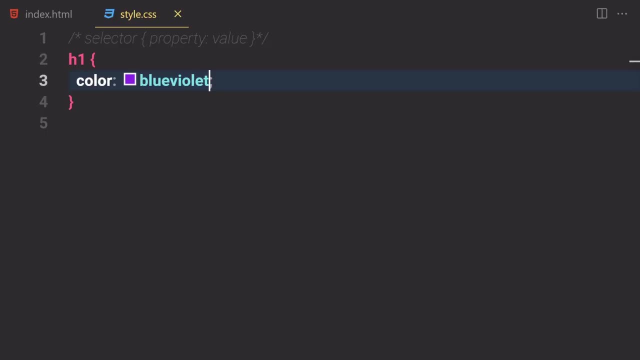 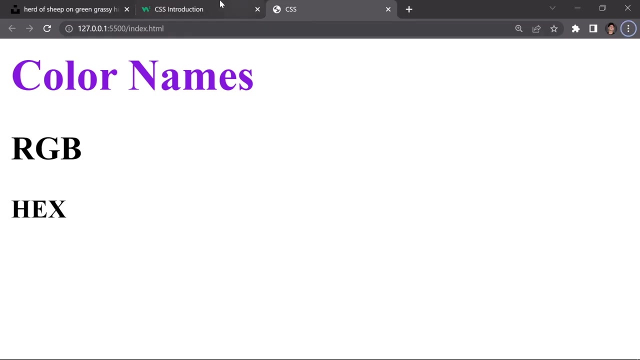 color right here, okay, so i'm going to you know i'm not going to close any of them, so this is the first way you can provide colors to it. now, the next thing i want to show you is something called rgb, and this rgb stands for like, red, green and blue. so to work with that, first of all, let me show you the h documentation. 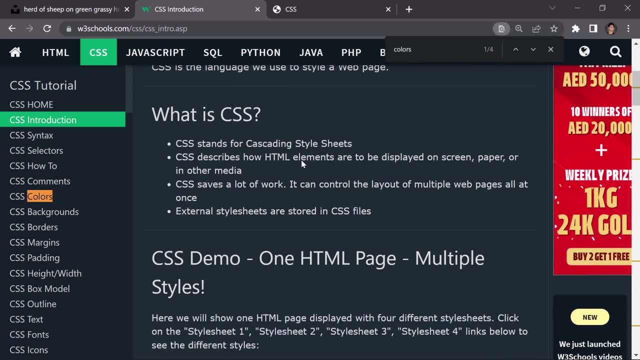 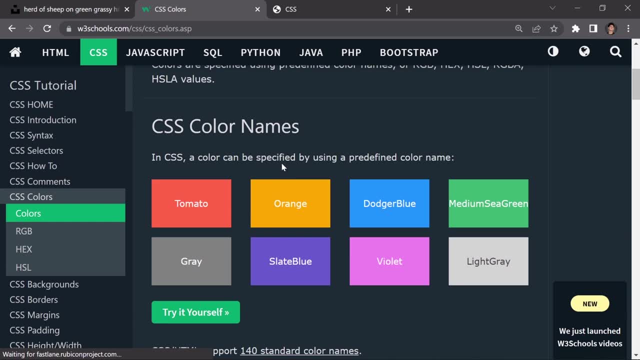 so i'm going to write like uh colors, uh in here. so we have a css color, so i'm going to click on that. um, i want to give you a documentation and stuff so that if you lost or uh, if you don't remember something, so that. 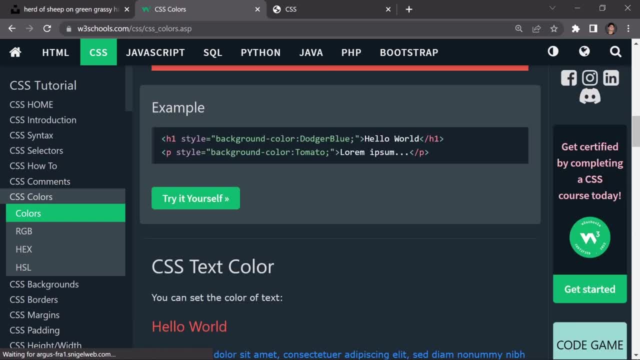 you can head back over through this stuff and you can learn more about that. so we have this color name, we have rgb, we have hex value and we have hsl and we are not going to be using hsl that much. like it stands for- like hue, saturation and lightness. this is useful for designer like those. 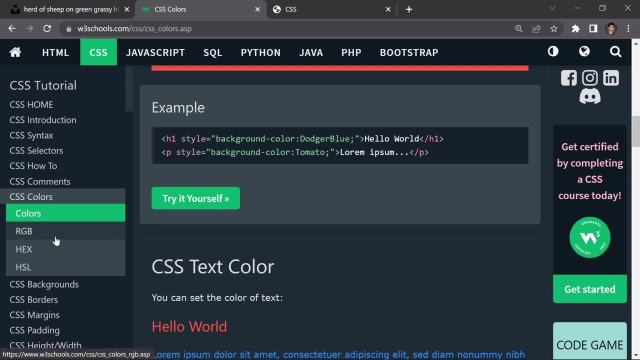 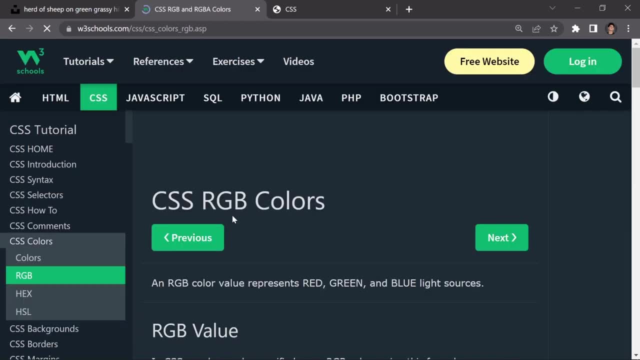 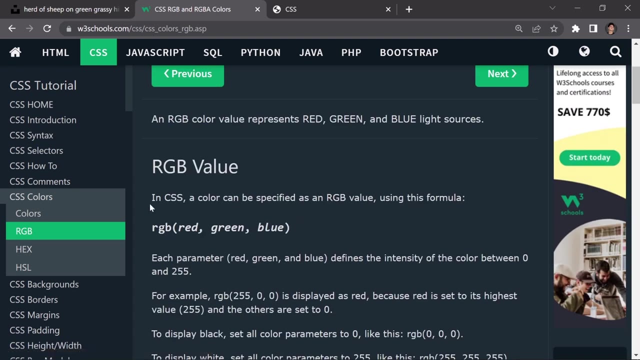 people who design the website, who don't code the website, okay, and these are also used for a graphic designer and stuff, but i will show you that anyway. so i'm going to just click on this rgb. so in rgb we represent red, as i said, green and blue- uh, lightness sources. so if you want to provide rgb, 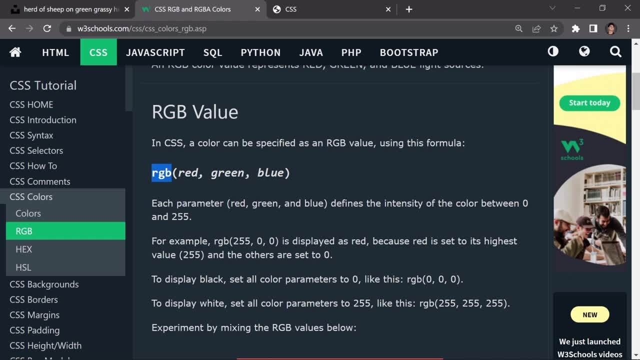 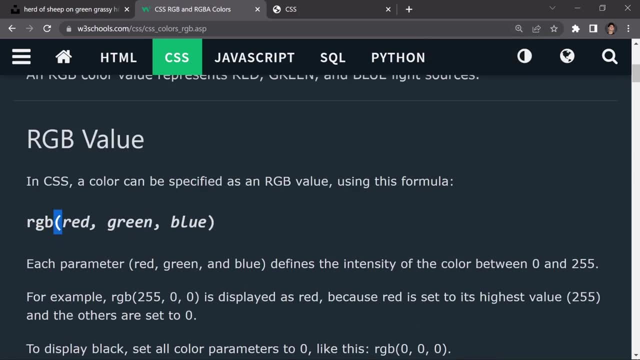 value. first of all, you just have to write this function, like you just have to write rgb as a value and then opening parentheses. let me just zoom in a bit so you guys can see everything: then opening parentheses, then closing parentheses, and then the first value will be for the red. 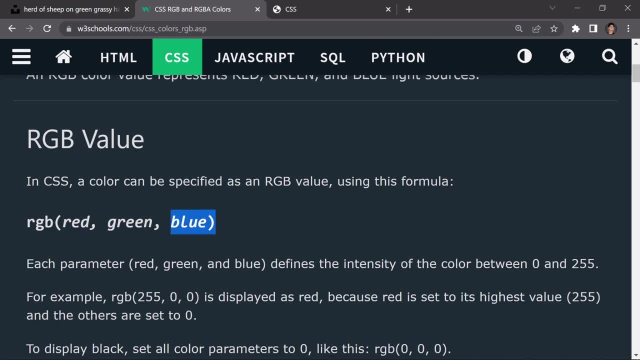 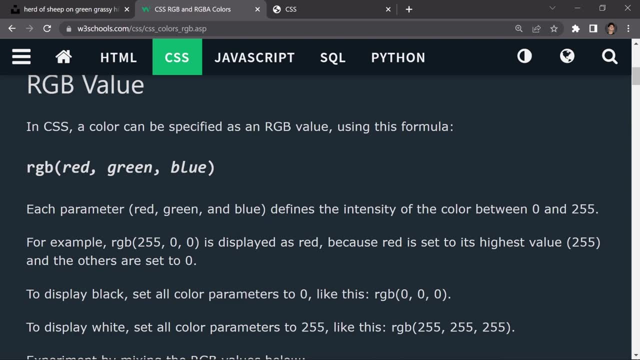 then the second value will be for the green and the third value will be for the blue one. each parameter- red, green, blue- define the intensity of the color between the two values, and then the two values will be set in 0 and 255. so zero will be the least value and 255 will be the top value. 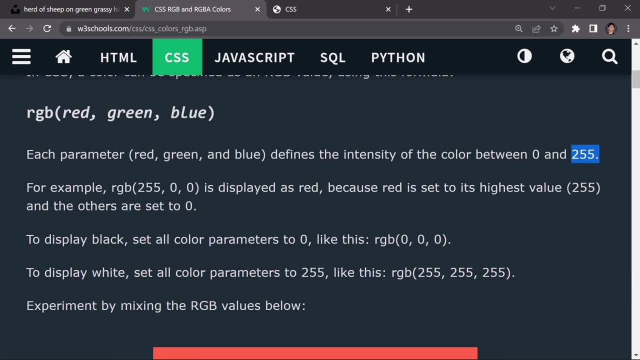 to display blacks at all. the color parameters to 0, like this: uh, rgb: 0, 0, 0. like red will be 0, green will be 0 and blue will be also 0. so what will we get? we will get totally black color and 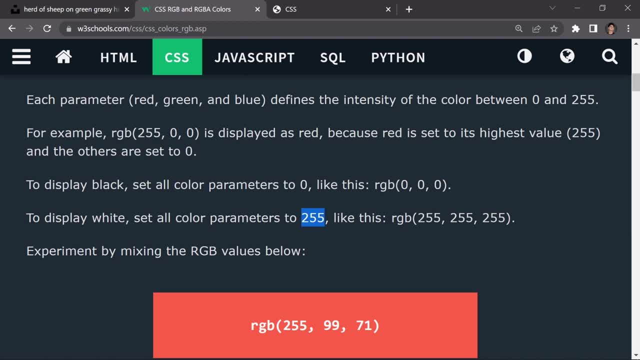 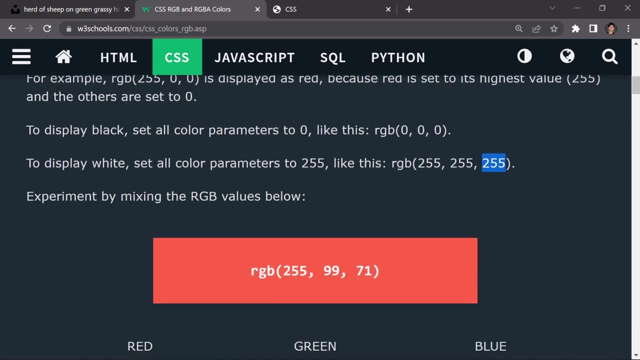 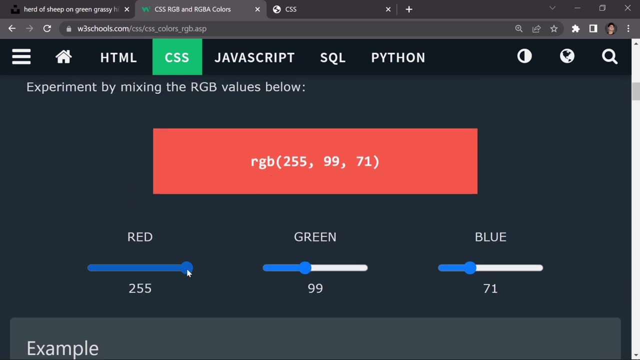 to display white. so you set all of the parameters to be 255, like rgb, 255 for the red, 245 for the 255 for the blue, red, green and blue and you can play around with that right here. so we are getting this kind of orangish color right here. that's because our red value is the highest right here. 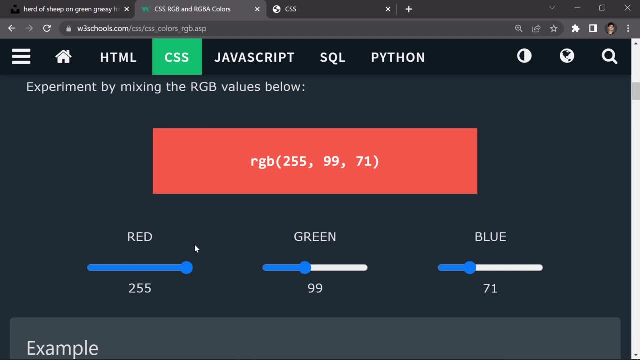 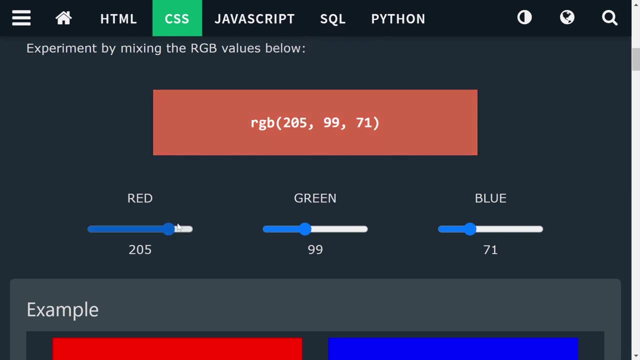 and i'm not going to go into a lot of math right here. it's not a mathy topic, to be honest. so i'm going to go with a presentation mode and if i just uh, decrease that, like, just focus on this color, if i just start to decrease that and now it become greenish and grayish and brownish and like so, 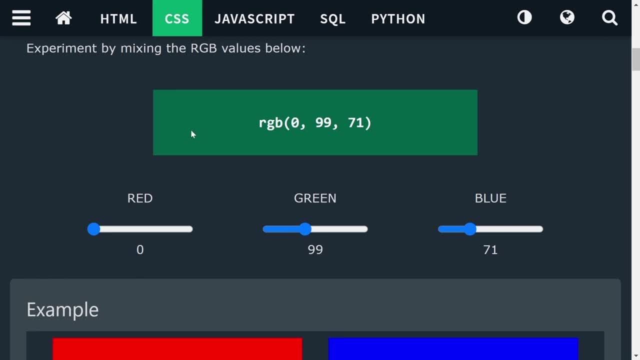 and now it's totally- not totally, i wouldn't say totally, but it's kind of a grayish green. okay, so if we set this blue one to totally zero, so what do we get? we get kind of a greenish color, as i said, kind of not a totally green if you want to get a totally green color. so for that we have. 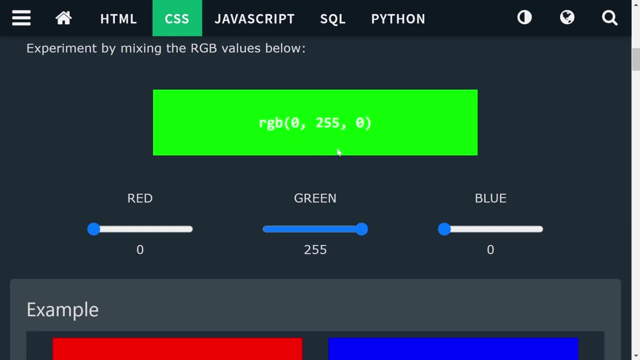 to bump it up. so here you can see, we get like totally green color. so now, here you can see the rgb. the red value is zero, the green value is 255 and, as we learned that 255 will be the highest value, and then we're going to set this blue one to totally zero, and now it's totally green. 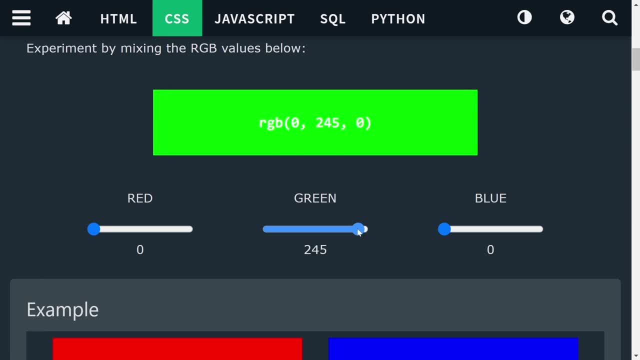 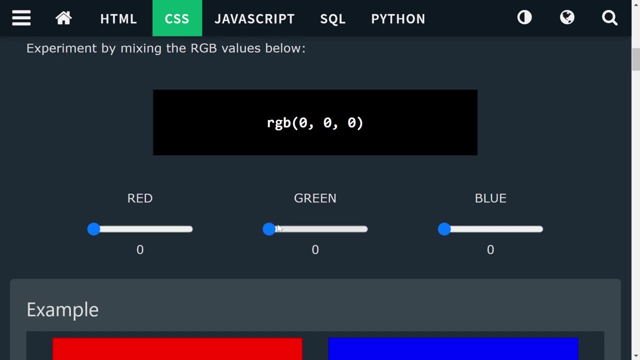 and we have our blue value, and blue is also set to zero. so that's why we get like totally green color. if you want to get like a red color, so we have to first of all set everything to zero and here you can see, it will not use this black and now if we bump up this red color. so here you can. 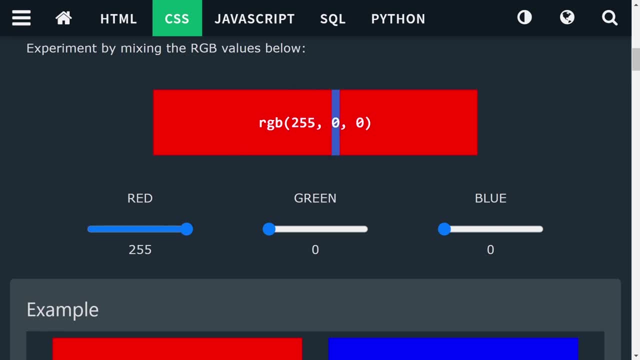 see, our value is set to 255, the green value is zero, blue value is also zero. so we get like totally red color and if we bump up everything so it will not use this totally white color right here. okay so, and, by the way, let me just 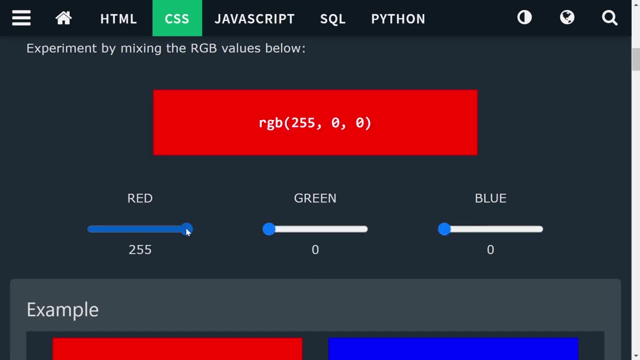 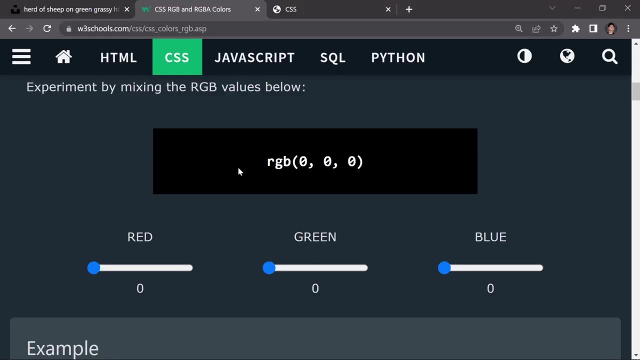 enhance your knowledge a little bit if you set everything to zero and it will give us this black color right here, and black isn't even a color, and a lot of people think like, uh, i love black color, like i love this black color t-shirt, and black is not a color. black is the absence of color. so if 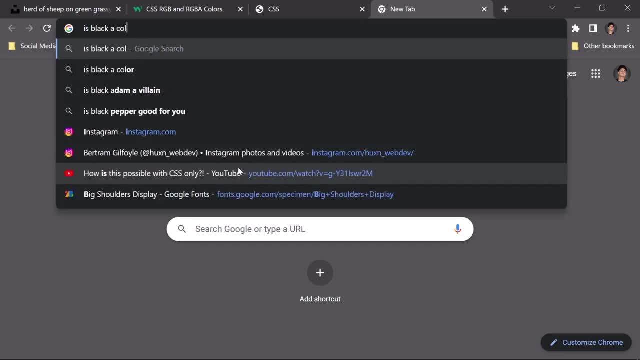 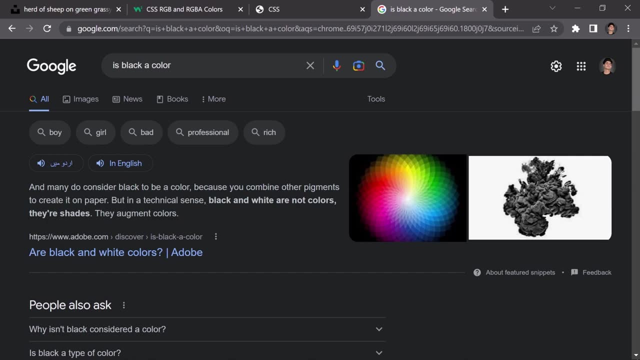 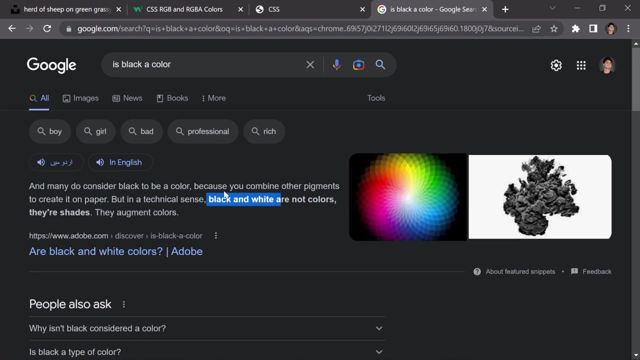 you search for um is black a color. so it will now give us this result: like- and many do consider that black to be a color because of the combination of the pigment to create it on a paper. but in technical sense, black and white, both of them are not even the colors, they are just the shades and 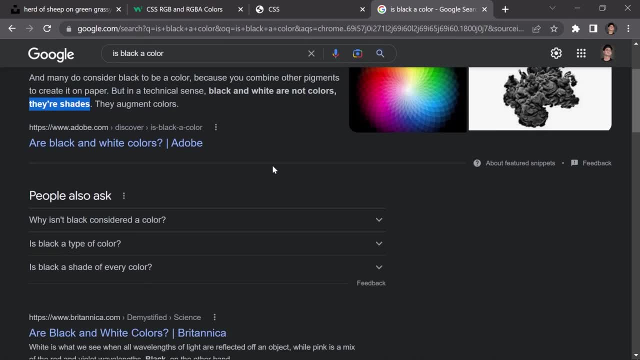 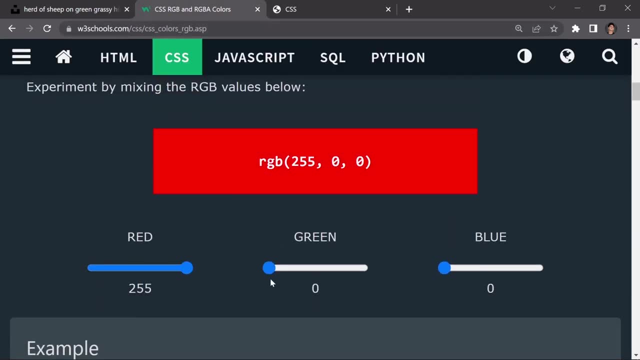 you are totally free to explore more about, uh, all of that. but i just kind of want to tell you, like black and blue, aren't you want to color? so i'm going to just cut there. and if you set everything to the white like, so i mean like set everything to highest value, so we would get like totally 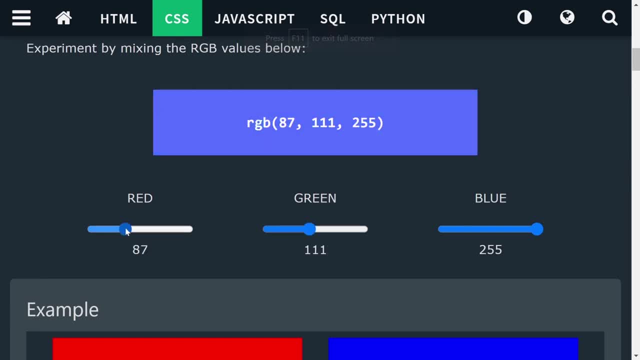 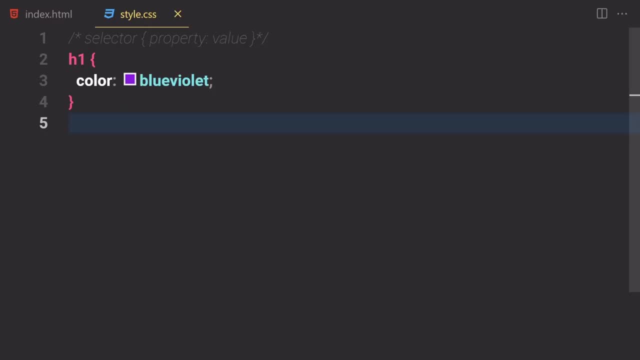 a white color and you can play around with these colors if you want to like- bluish, kind of reddish, kind of uh colors. so now let's jump into our coding. and now let's just start working on our coding. so now, if i want to select this h2, so what do i have to do? i'm going to go to my css and i'm going to write like h2 and 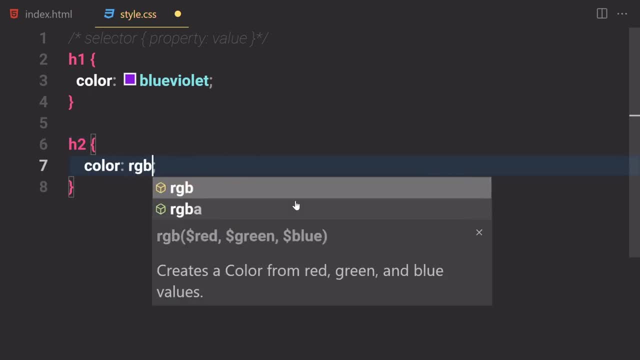 here i'm going to just write like color, i'm going to write rgb and if i hit tab, certain log uses these parentheses and it will also give us like red, green and blue. okay, so i'm going to just provide like 255 for the red value and if i hit tab and i'm going to write like 0 for the green, 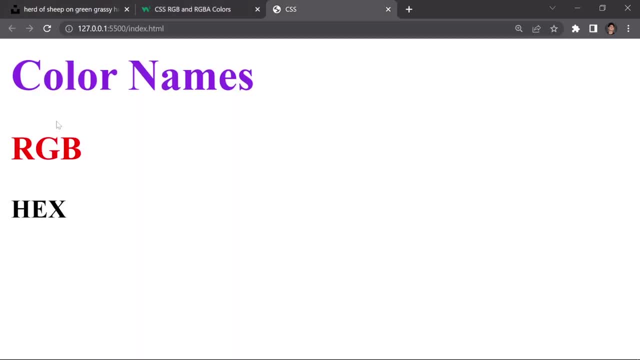 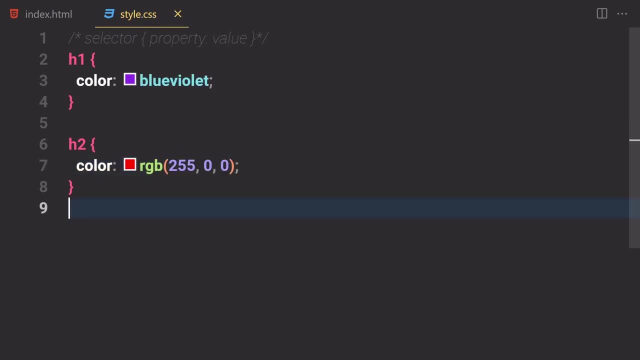 and 0 for the blue. and now if you save that- so here you can see, the log uses totally red color right here and now. if i just set this to- let me just come on- if i set this uh red value to zero, and if you set this to like 255, and if you, 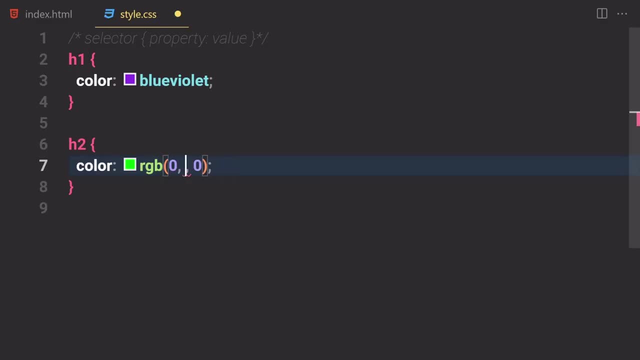 save that and here you can see, the log uses, uh, green color. if you set that to zero and if you just write 255, certain log uses blue color and you can play around with that, like if you just write like 40 and then 10 maybe, or yeah, 10 would be fine and we'll just 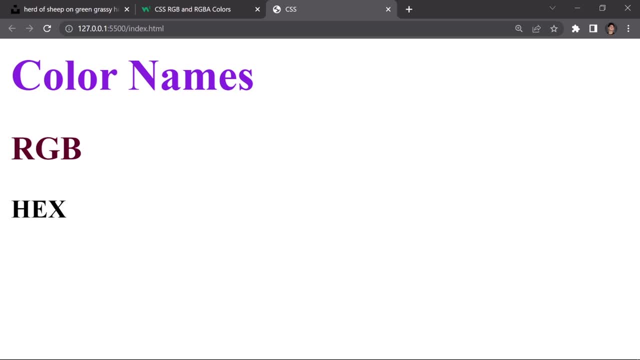 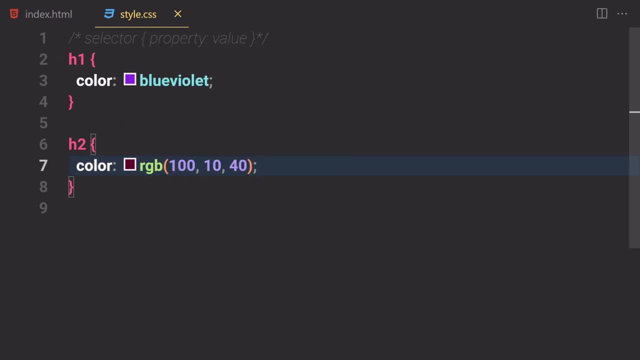 and then let me just write 100. so if you save that, it will give us kind of a creamy color right here, kind of a creamy red color, and you can play around with that. and, by the way, let me tell you one more thing about a visual story quarter. so if you hold our mouse over to this color, and here you- 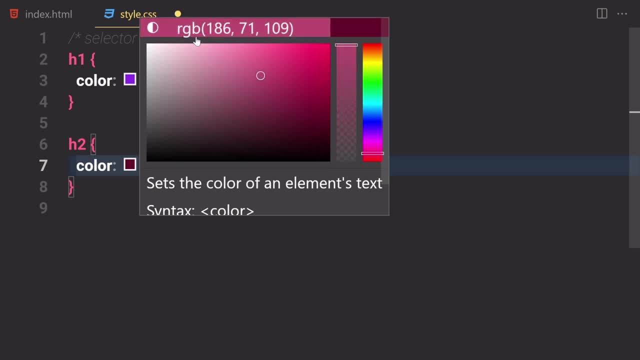 can see. we have this color picker right here. we can change the color here. you can also see that this rgb values and if we can change the color from here, like this is kind of a tealish color, we have kind of a greenish color and kind of a brown. 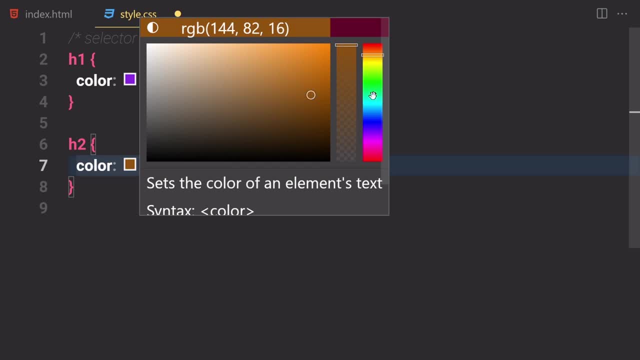 brown, coral or chocolatey color, whatever you want to call it. so I'm gonna set this to RGB value and if I click on this RGB- and here you can see- it will also give us a hex code right here and which you are going to be exploring just in a second. so if you click on it one more time it will give us. 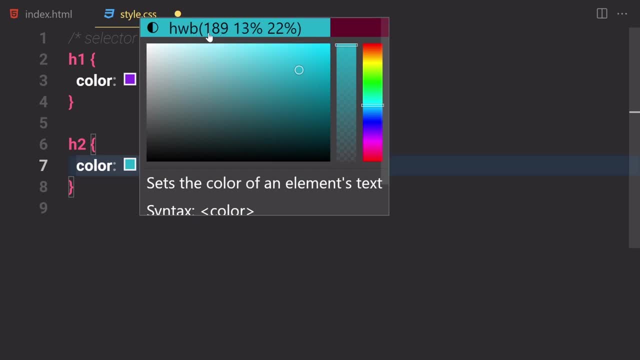 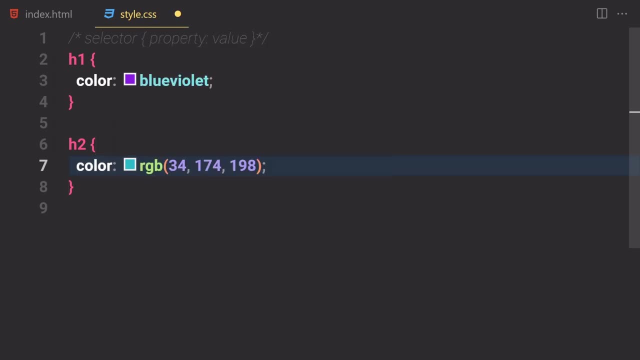 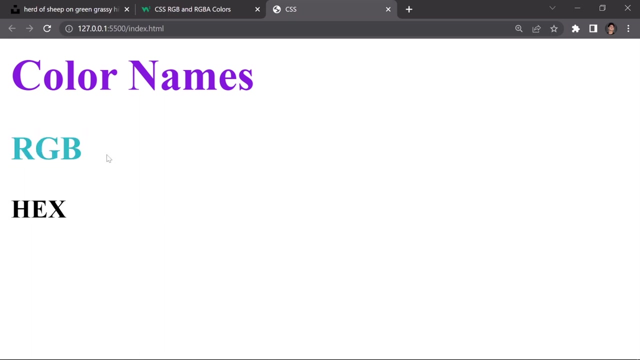 the HSL code. and then hwb- excuse me, I've never used hwb in my life, so I can say something about hwb- and then we have RGB. okay, so let's suppose if I choose this color and if we save that, and what do we get? we get this tealish kind of color right here. okay, so this is. 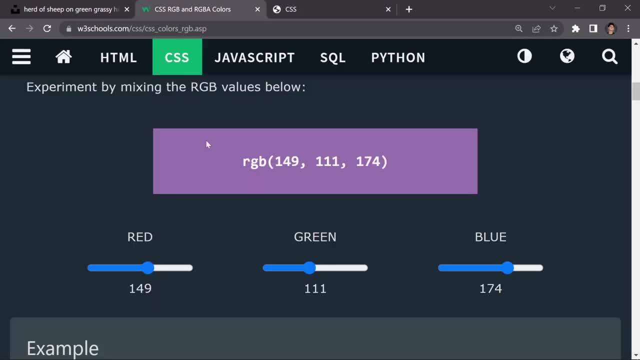 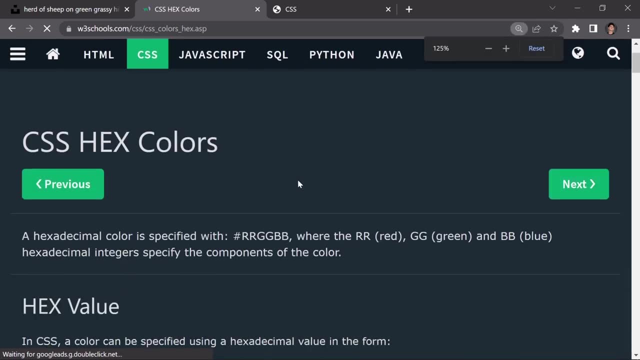 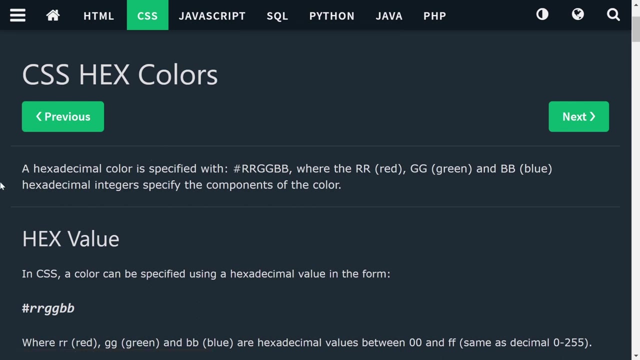 looking awesome. so that was it about RGB. now let me just tell you the last one- or not a loss on, we can still have to call the HSL, but I'm gonna click on this hex one and this is my favorite one. and a lot of developers and a lot of designers still- uh, I shouldn't have to say still, but are 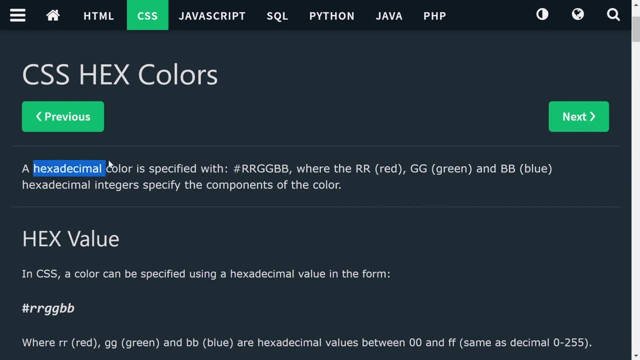 using this hexadecimal. these are my favorite hexadecimal is my favorite one. so hexadecimal color: g, g, b, b like red for the r's, g I mean like green for the g's and b for the blues. okay, where the r is red, g's are blue. uh, g's are green and b's are blue. hexadecimal integers specify the component. 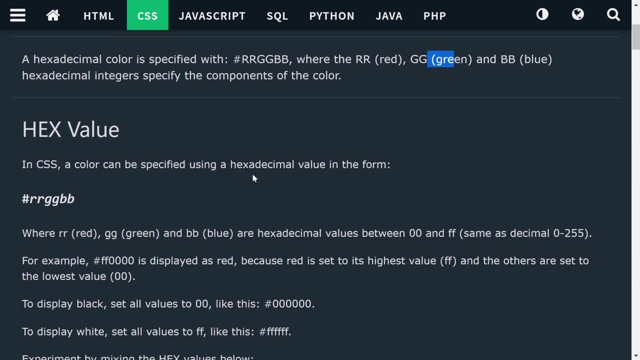 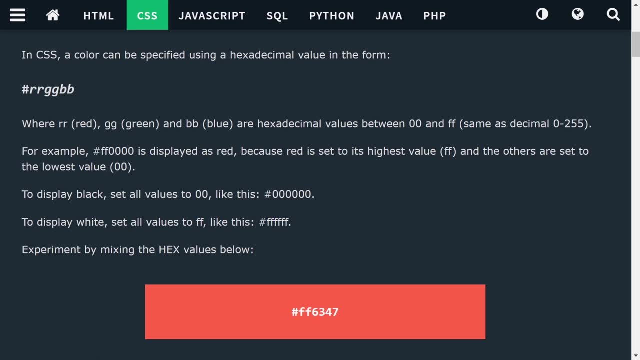 of the color hex value. in CSS, a color can be specified using a hexadecimal value from r, r, g, g, b, b, where r is red, green and blue. hexadecimal zero between zero- like zero, zero will be the least value and f- f, it will be the highest value, same as the decimal from like zero. as we saw, like RGB values, RGB was. 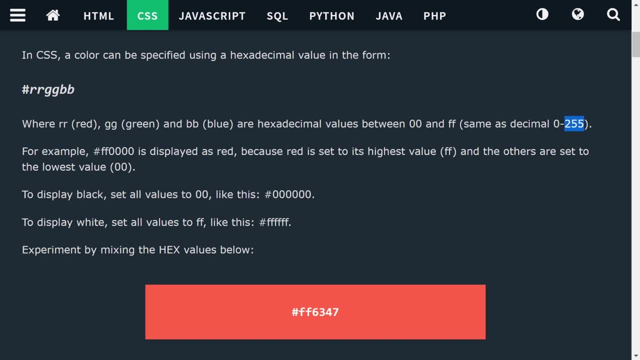 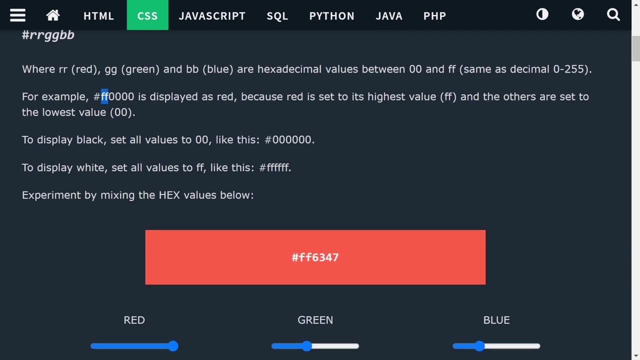 like zero was the least value and 255 was the highest. so now in the hexadecimal the 00 is the least and FF is the highest value. for example: uh, FF. so it will not use red color because we just provide the first value, like the rr value to be the top. so it will not use a red color. so FF is. 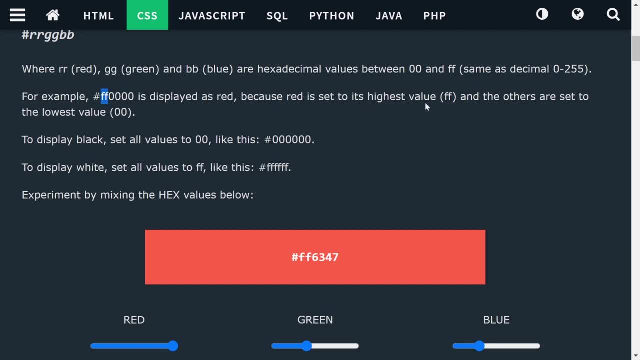 uh displays a red. uh because red is set to its highest value, FF and its other are set to the lowest value. like zero, zero to display black color. set all of the values to like zero, zero. and here you can see we have six zeros like um. two zeros for r are red, two zeros for green and two zeros for blue. okay, and you can. 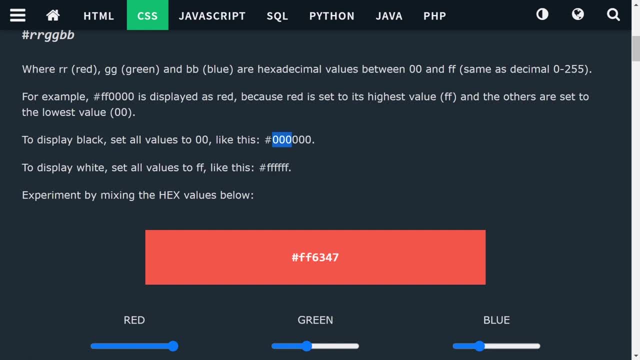 just write like uh, three zeros, uh. it will also gives us like black colors, uh, black color, like um red, green and blue, if you want to work with that, uh, six F. so it will also give us totally white color, but we can still go with three F, so it still. 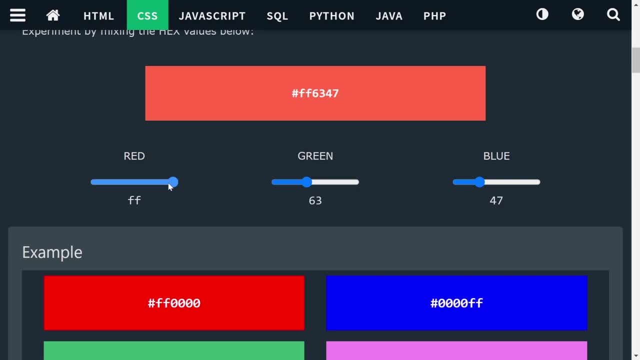 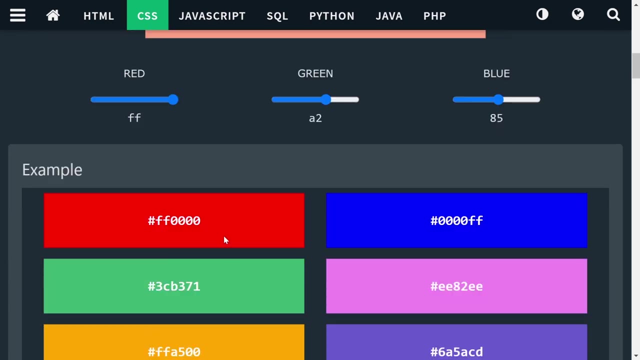 gives us like white color, and here you can see, we can play around with that by just um, making it smaller or lowering or hiring, like so I don't want to go into the details of that- and you can also write letters and you can also write a numbers if you want to. okay, so now let me just show you all. 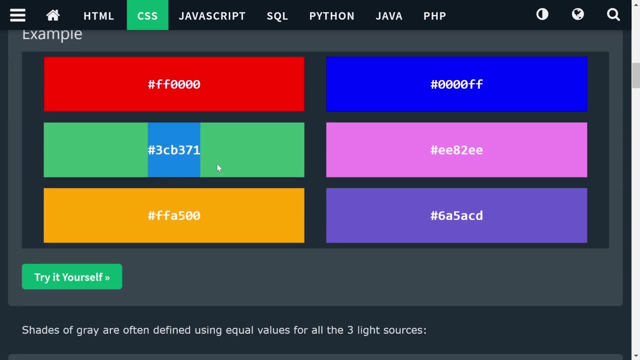 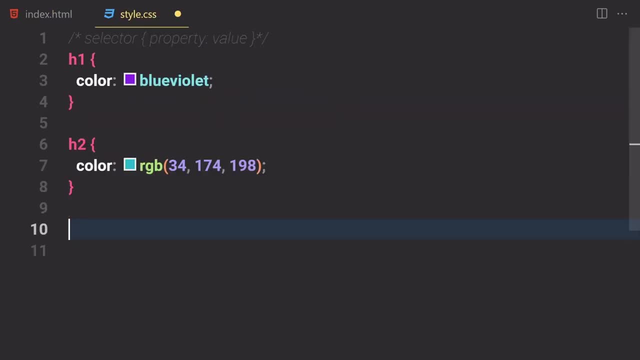 of that in code. and now here you can see my favorite color, not my top favorite color, but just a little bit favorite color. all right, so now, if you want to select this H3, so what do we have to do? we just have for H3 in here and here. I'm going to write a color in here and I'm going to paste. 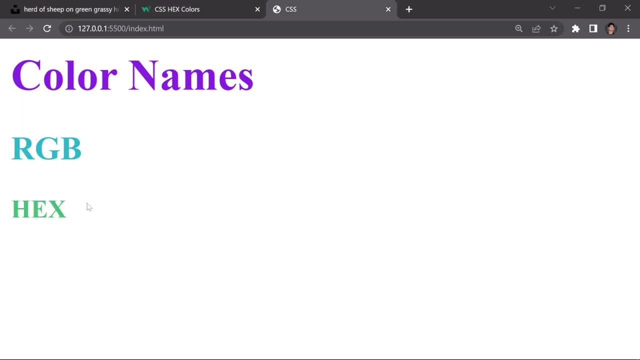 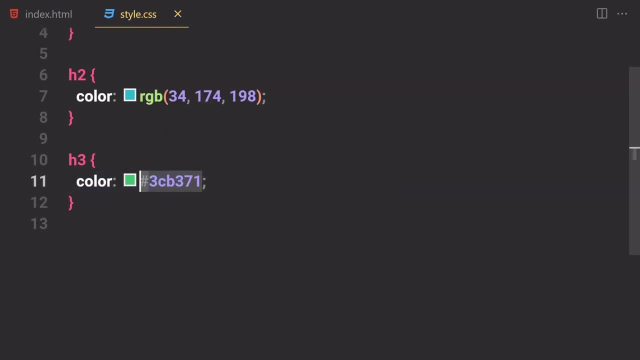 this color. so I'm going to save my file and here you can see this become. do that, uh, kind of a greenish color. and by the way, I forgot to mention one thing: if you want to work with a hexadecimal value, first of all you have to provide this pound symbol, or hashtag, whatever you want to call it. so 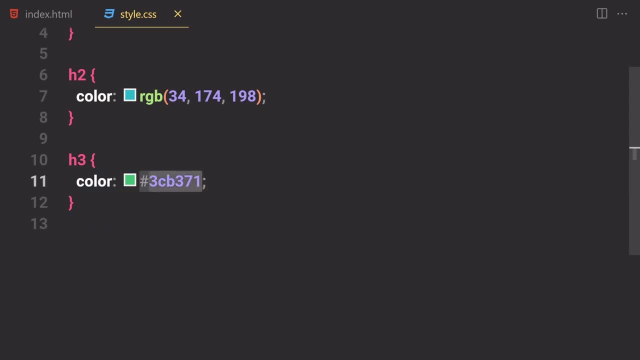 first of all you have to provide that and then you can provide, uh, the other numbers and stuff. you can play around with that. so in my case, we want to work with the red color, so I'm going to just write like FF and zero, zero, zero, zero. okay, so this is a red color. 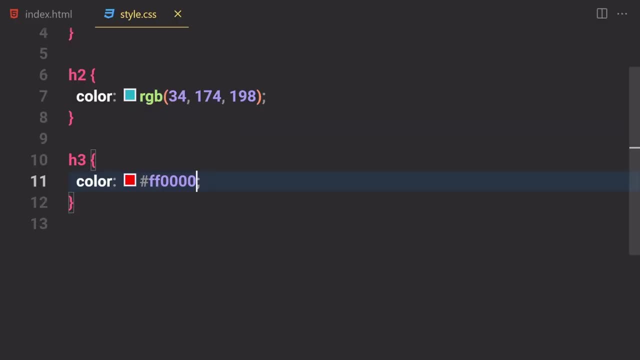 if you sell that, and here you can see we get like totally red color, if you want to get like kind of a blue color, like totally blue colored. so first of all you're going to be writing zero, zero for the red and then like FF for the blues if you sell the actual. okay, so red, green, my bed. so this is zero. 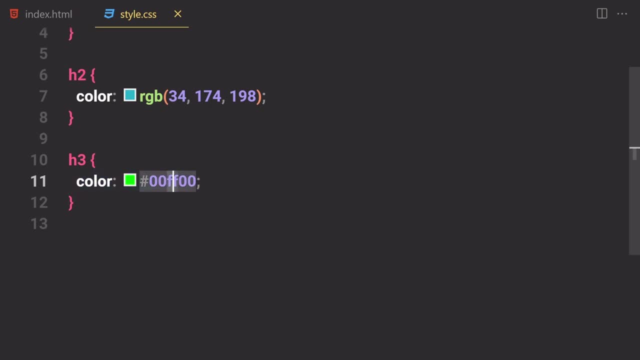 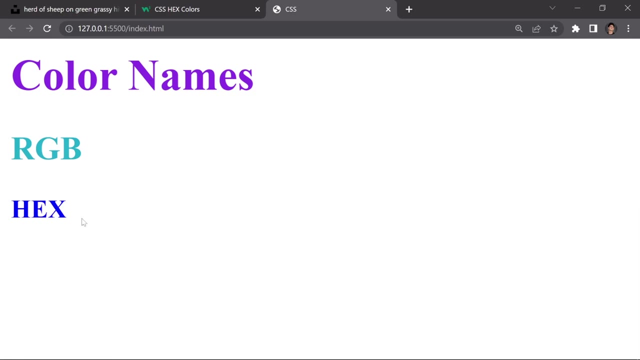 zero. I mean, like, this is the greenish uh shirt, so I'm gonna just write zero, zero for this one. and finally we have a blue one. so now, if you sell that, and now here you can see the log uses like blue color right here and you can play around with this color. so if you just click on that, and now here you, 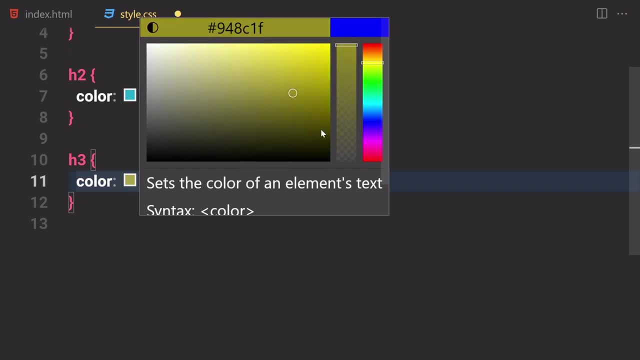 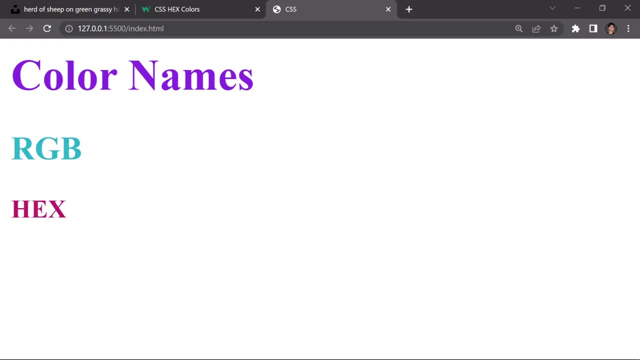 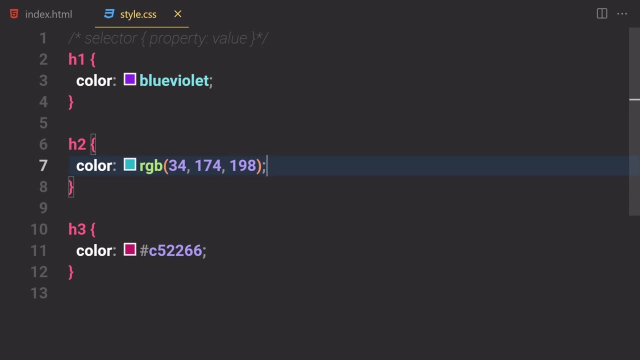 can see, we can change the color. you can change it from here, like so, if I, let's suppose, if I want to change this color to this kind of a creamy Crimson color, so if you sell that, everyone uses this color right here. and, by the way, I forgot to mention something called RGBA. so now we learn about RGB, which stand for like red, green. 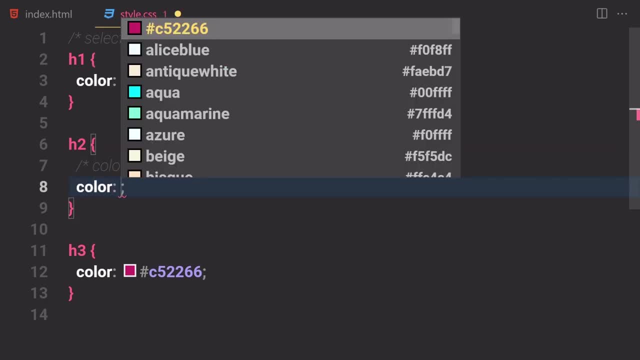 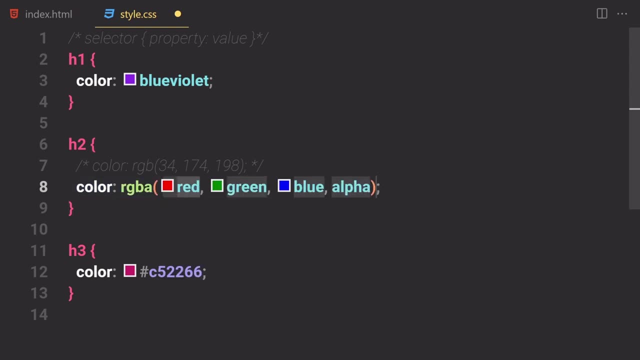 and blue, and we still left with one other so, which is called RGBA and a stand for Alpha transparency. so we have RGBA- red, green, blue and Alpha transparency, so we can just write like 255, then we have zero, zero, and Alpha transparency will be like 0.5 in this case. so first of all, let me show. 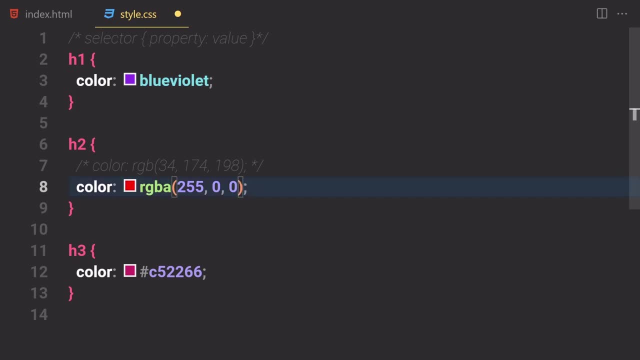 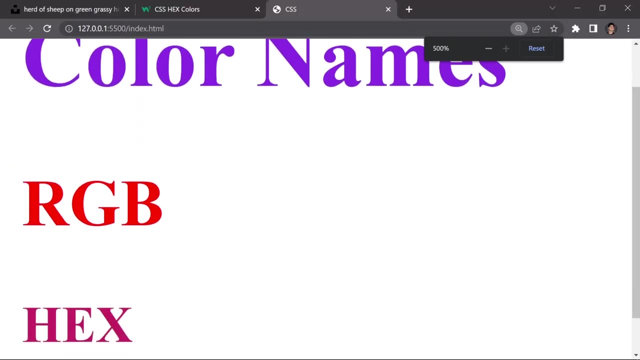 you that without Alpha transparency- and then I'm going to show you a little bit of Alpha transparency- so if you sell that, and here you can see, it will not use a totally red color right here. I want you to just focus on this red color. and now, 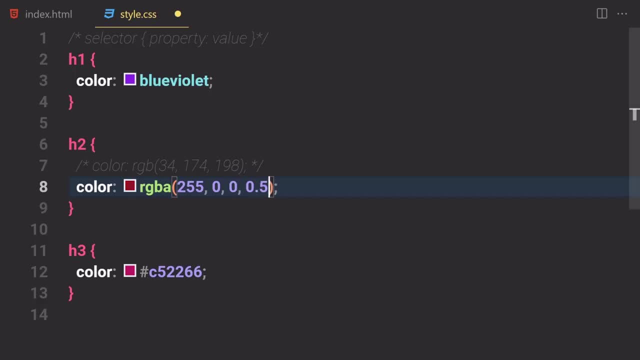 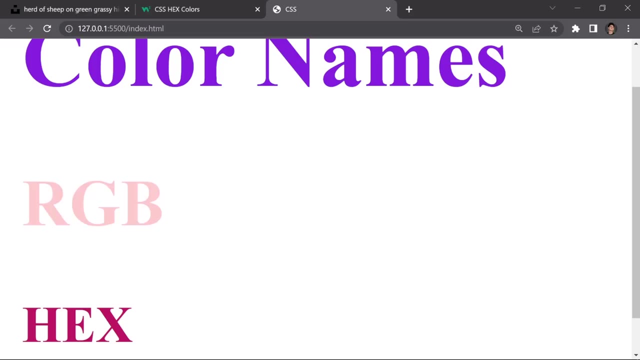 if you just put a little bit of Alpha transparency, like 0.5 maybe, and if you sell that, and here you can see it will not just put a little bit of opacity to it, like 0.2 would be fine, and here you can see it is now making it subtle like so okay, so we can also change the opacity or transparency. 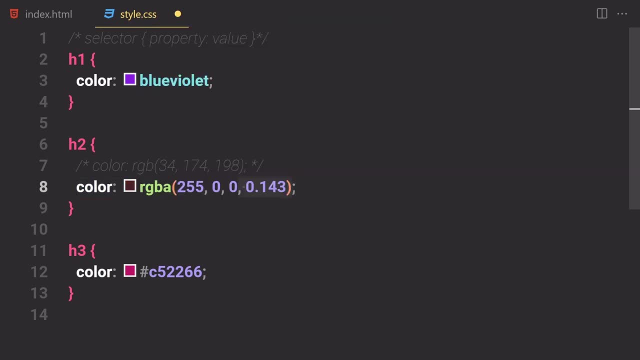 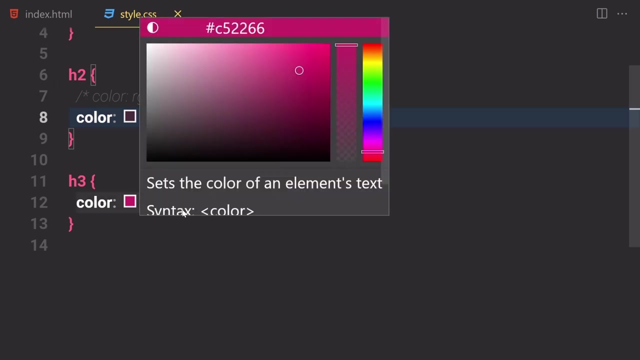 to 0.1 and we can play around with that, like we have 143. and now if you save that and we can really see or text right here, and this can be handy in some situation, but not in the majority of them. and now if you're wondering, like how can I change the hexadecimal transparency so you can just click. 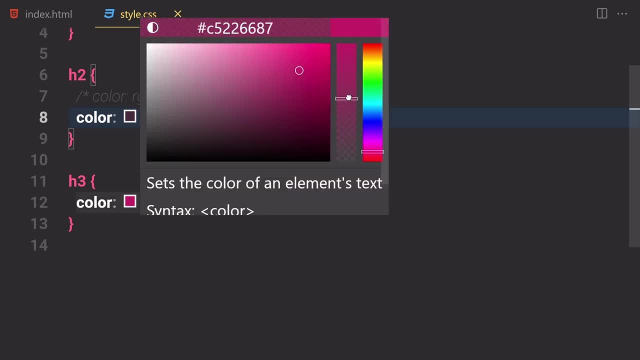 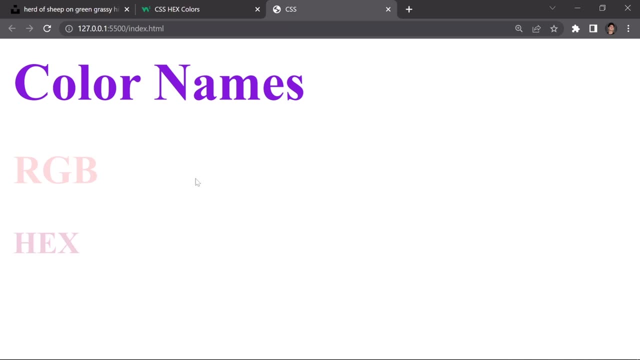 on that and then you can just change the its transparency from here right here. okay, so in my case I'm going to just go with lowest one, like so, and if you sell that and this is how it looks like I've already done with the colors, but I just kind of want to give you the bonus HSL. I didn't plan to. 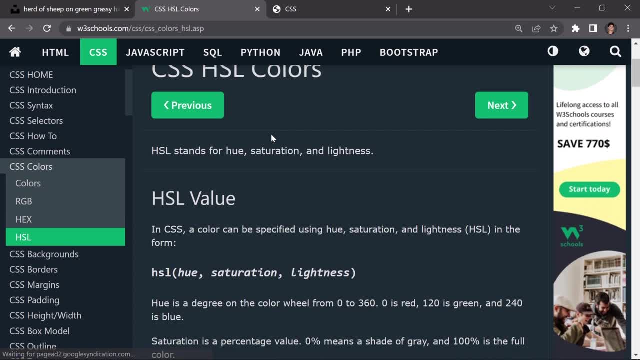 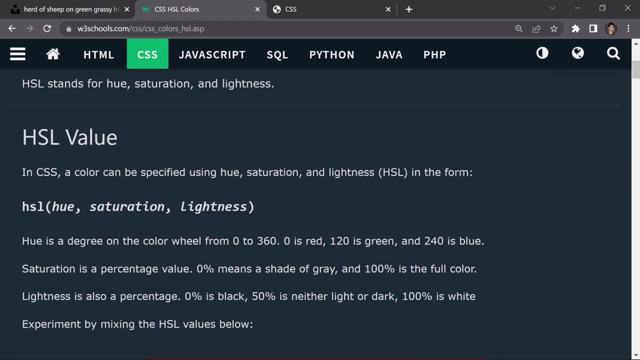 show you the HSL because it's a little bit weird so I don't want to include in my course, but I just kind of want to show you because we already saw that anyways. so HSL just stands for, like, hue, saturation and lightness. in CSS, a color can be specified using a hue, saturation and lightness. 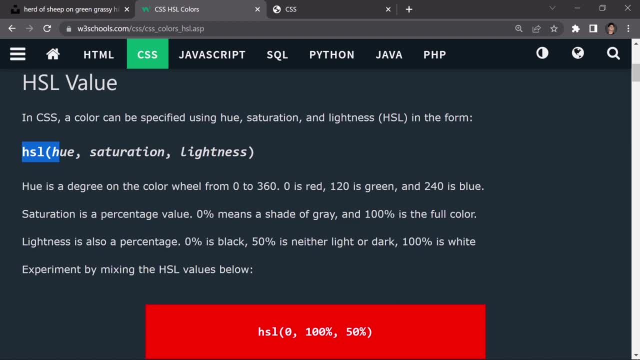 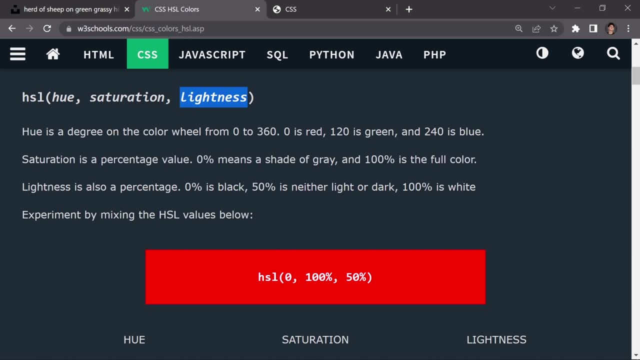 HSL in the form of this: like you just have to pass this function like HSL: first of all the hue value, then the saturation value and then the lightness. here's a degree on the color wheel from zero to 360, and zero is the red and 120 is a green and 240 is a blue. saturation is: 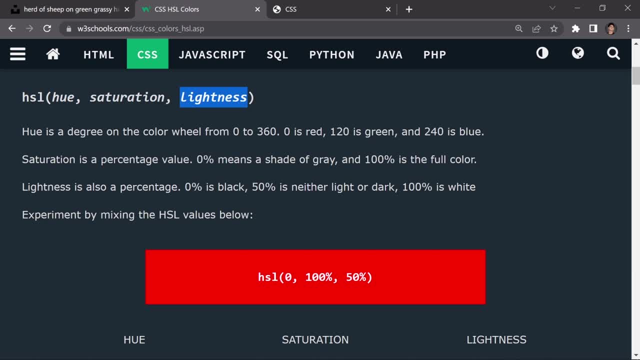 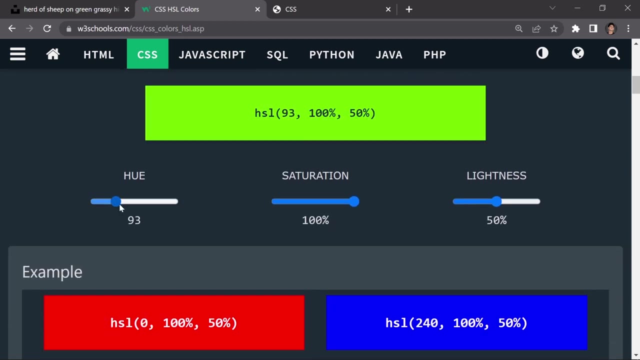 a percentage value like zero. percent means a shade of gray and hundred percent is of the full color, like the totally bright color. light is also a percentage and zero is black. thirty percent is neither light or dark and hundred percent is totally white. okay, so experiment by using these mixing values so you can learn more about that. suppose, if I want to provide this color. 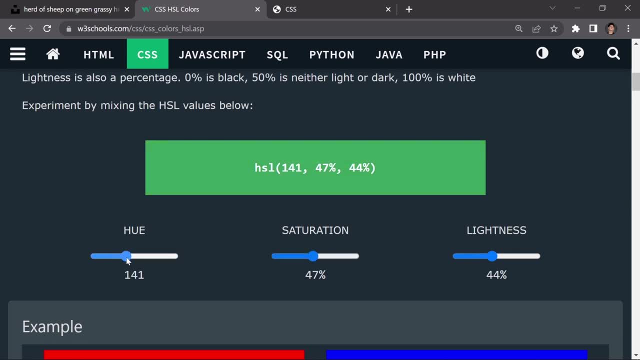 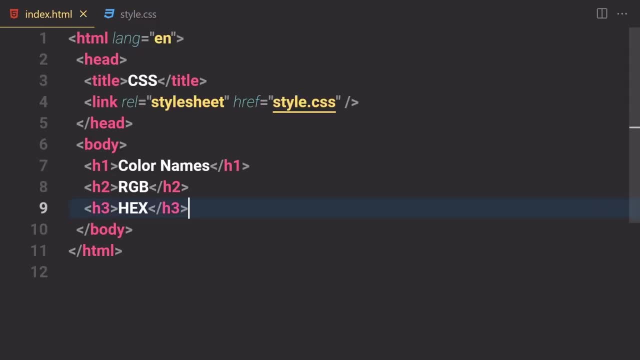 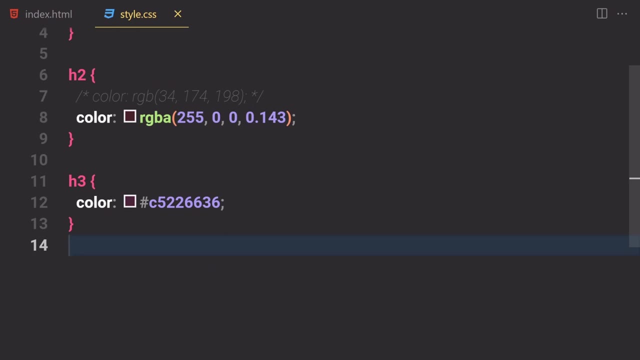 like so kind of a greenish color. yeah, I guess I would. that would be fine. so you just have to copy that and then just uh select, like let me just provide HSL in here, H4, H, uh, SL, hue, saturation lightness. and now let me go to my CSS file and here I'm going to just write H4 and here I'm going. 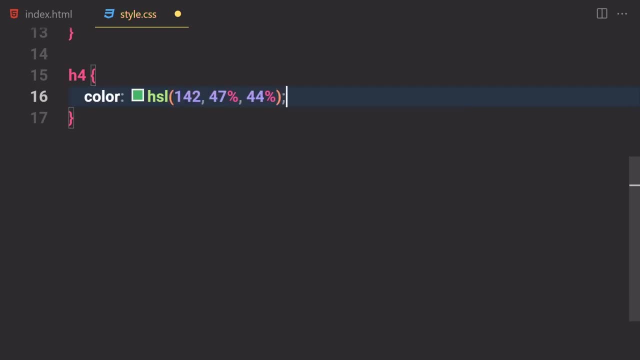 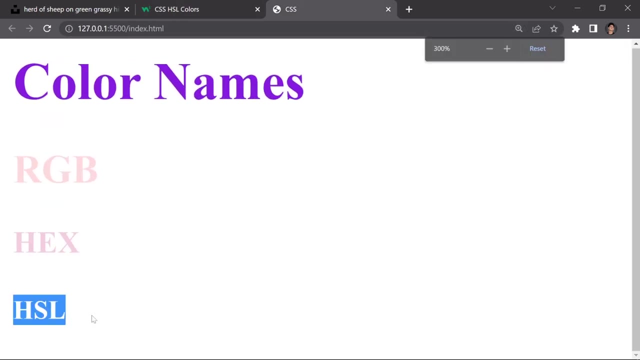 to pass it. okay, I have first of all write a color and I'm going to paste it right here. so if you say on there and now if you go towards CSS file, so okay. so here you can see that it's a cell right here. it's kind of a greenish color, okay. so we are. 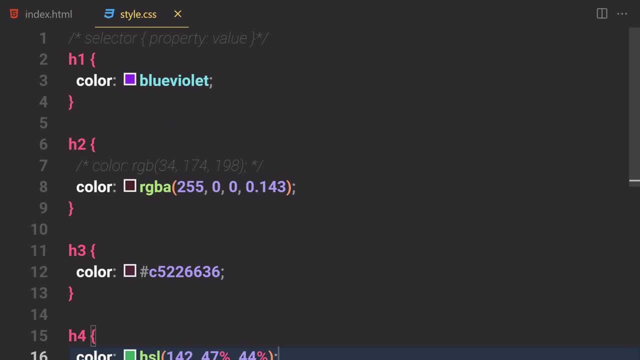 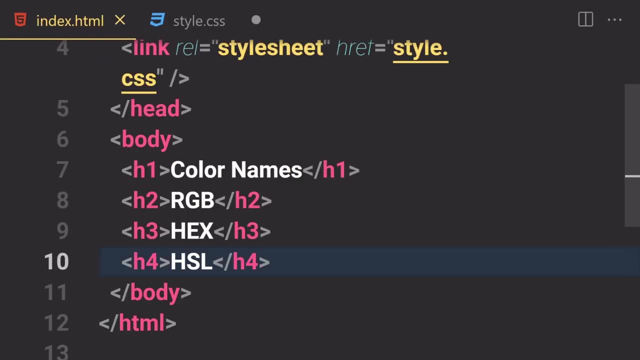 totally done with uh or color properties. so now let me just show you one more color property which is a background color. so I'm going to just remove that. and now suppose, uh, I wanted to get this. you know, I'm going to hide this meta or head area. I'm going to remove this, everything, and I'm just uh. 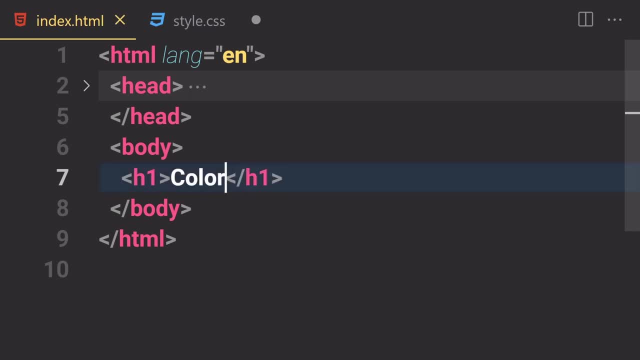 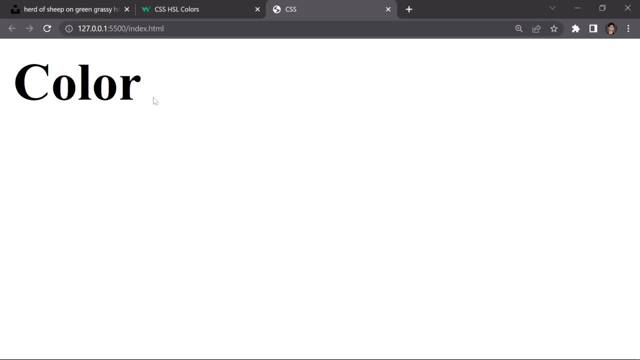 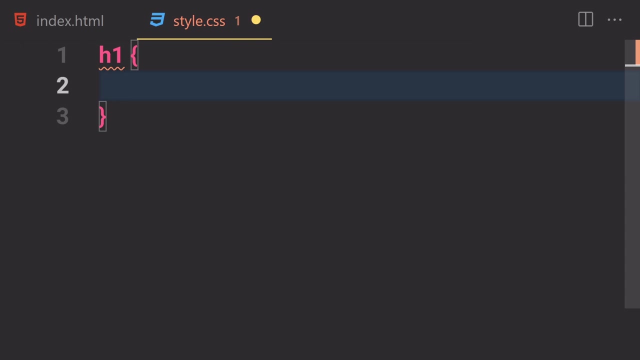 left with this H1 of color names. I'm going to just write color inside there. so we just have one H1 inside of our property, right here and now. if you save that and we have totally black, okay, so if you want to change the background color of this H1. so what do we have to do? we have to first of all select this H1 and 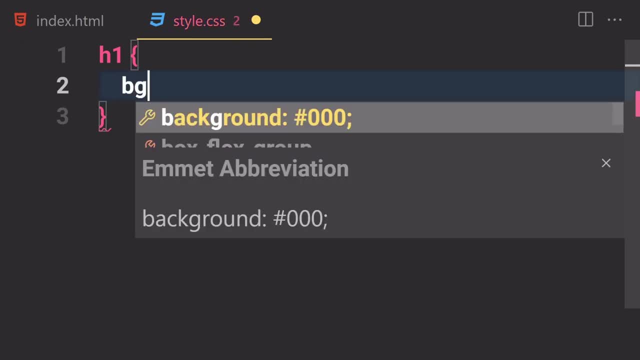 instead of writing a color, we can just write, in this case, a BG, and if you hit tabs it will give us this: uh, by default black color. but we can still write a background and then color. okay, so we can just provide a color, like we can use HSL, RGB, hexadecimal or even a color names. so I'm gonna. 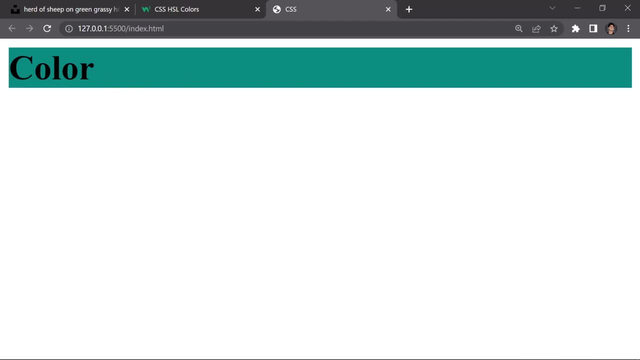 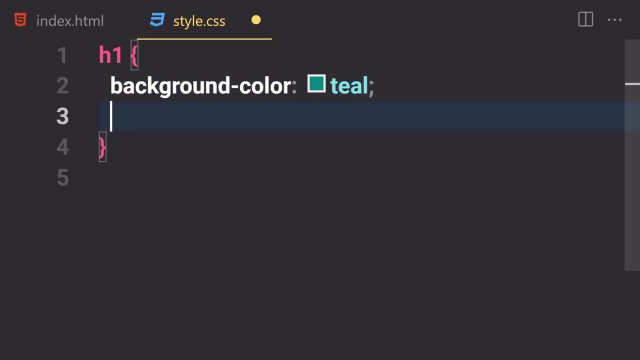 say so. if we save that and here you can see, it'll now just change the background color of this text right here: H1. and now. if you want to change the text color to be like white, so we can just write like color and totally white, okay, or we can use the pound symbol and totally FFF. and now, if you, 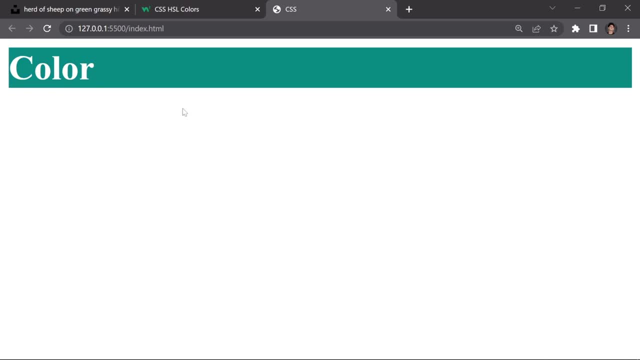 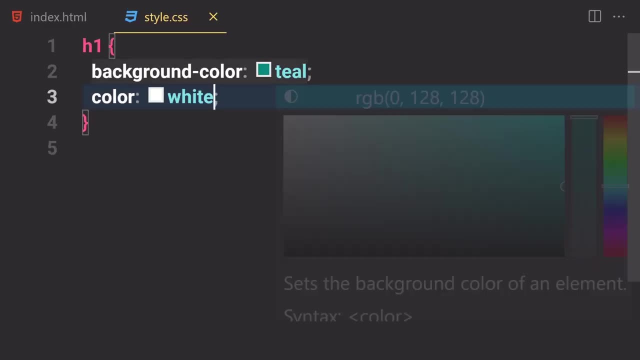 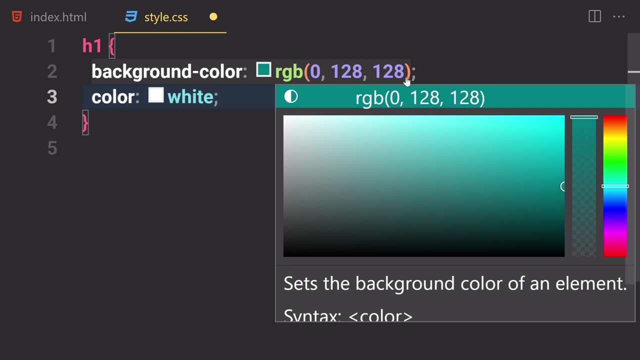 save that. and now, here you can see, the color is now changed to totally white. okay, so we can do a lot of crazy stuff with uh. like, let's suppose, if I want to provide uh, HSL or RGB value, if I just click it will not give us that HSL, HWB, RGB. okay, so we can play around with that if you want to. 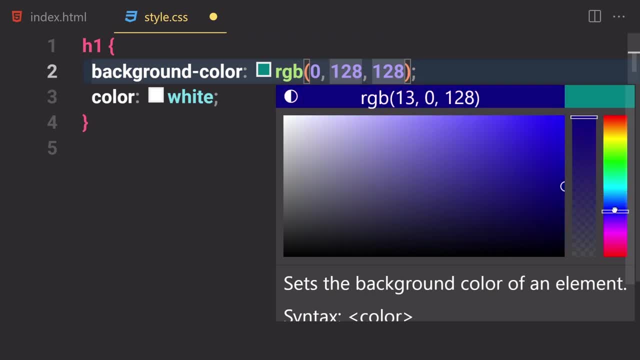 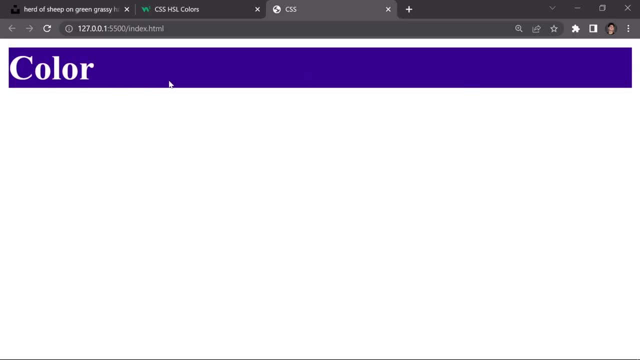 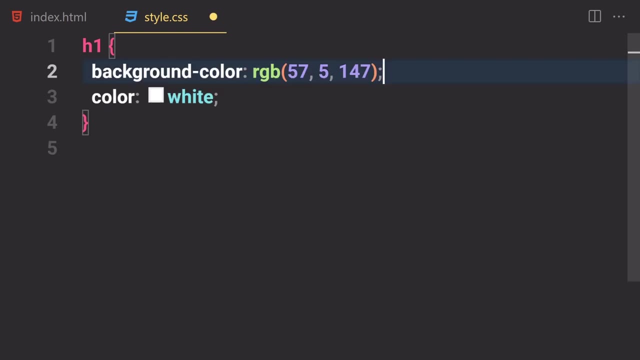 click on here and somewhere click on select kind of a bluish color or you know what, blue, violet color will be fine. so now, if you select that and if you save it and this kind of a blue, white color right here and we can remove that, boom, okay. so now let's just stick to. you know, I'm gonna just 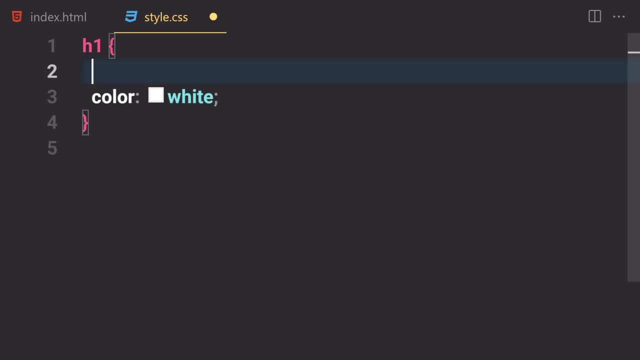 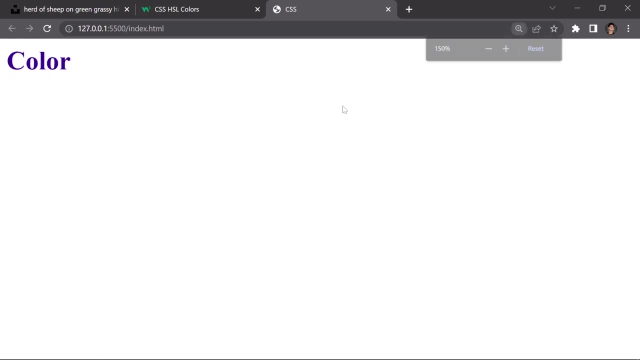 get this blue white color from this one and now save a bite background color. I'm going to remove this white color. I'm going to paste this blue wire color right here. so save that and boom, and this is how it looks like. okay, so we learned enough of. 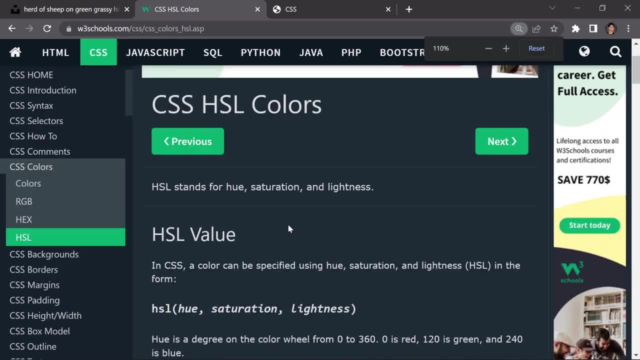 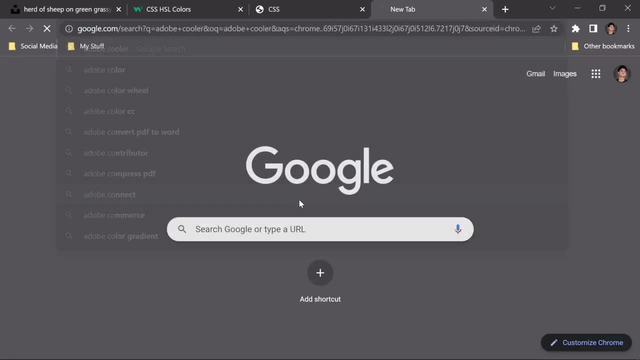 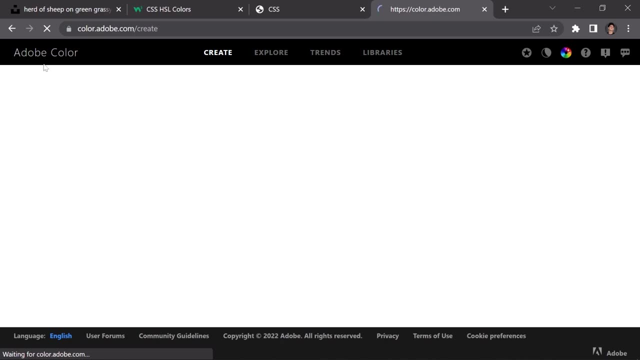 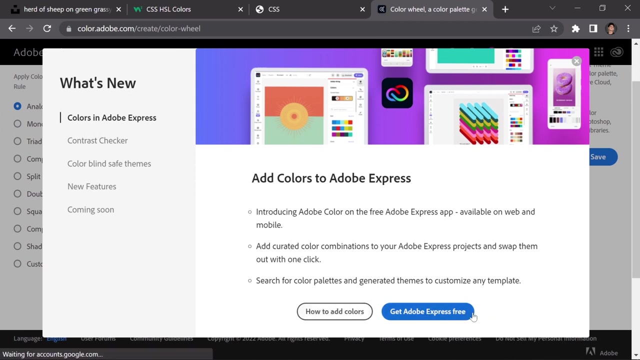 we learned enough about um CSS colors, so now let me just show you where to find great colors. so Adobe cooler: c double o l e r? um, it used to be Adobe k o w e r, but if you click on that so color, it used to be Adobe k double o l e r. uh, get Adobe experience for free. uh, how to add colors now click. 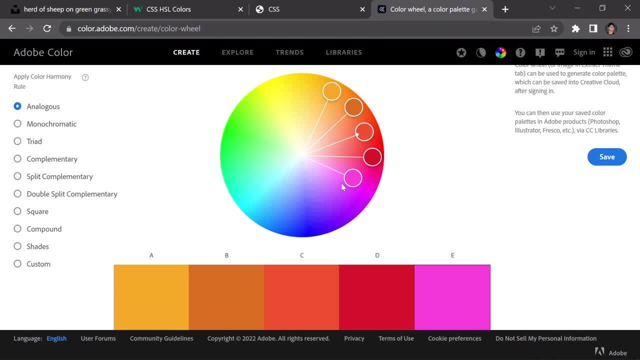 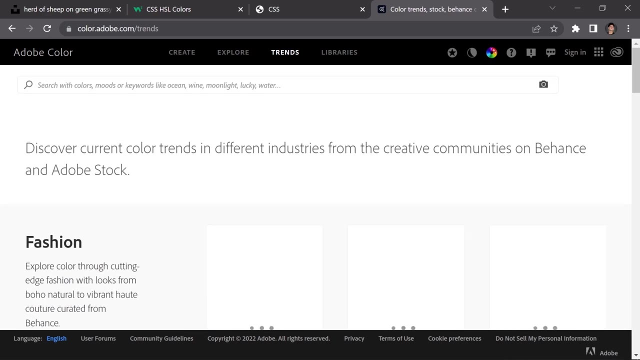 on this one, and here you can find a lot of great colors. if you want to like, you can create your own stuff. you can also click on this Explorer, or you can also click on this trendy one. so if you click on the trends, it will take a little bit of time. just wait for it. okay, so it will not give us a. 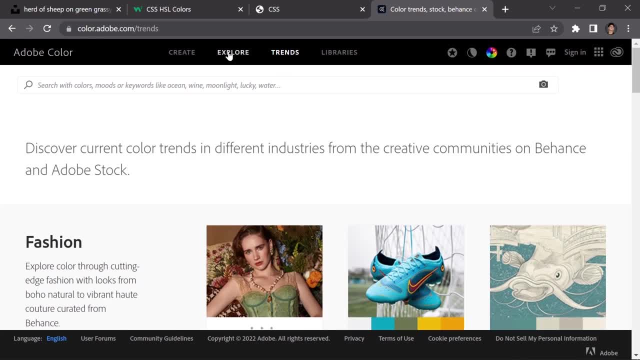 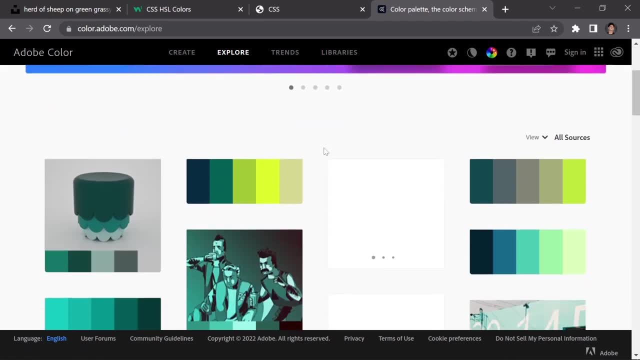 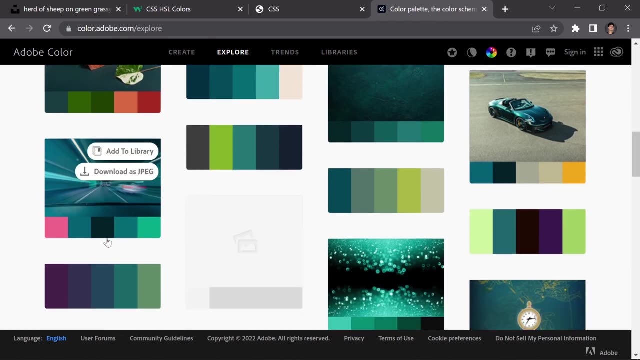 trendy colors. oh my goodness, not friends. but click on the Explorer and then go to trends. oh my goodness, uh-huh. certain log uses this uh kind of colors right here. you can choose a lot of different kind of colors from here. if you wanted to, maybe uh would just click on. you can download that or you can add that to. 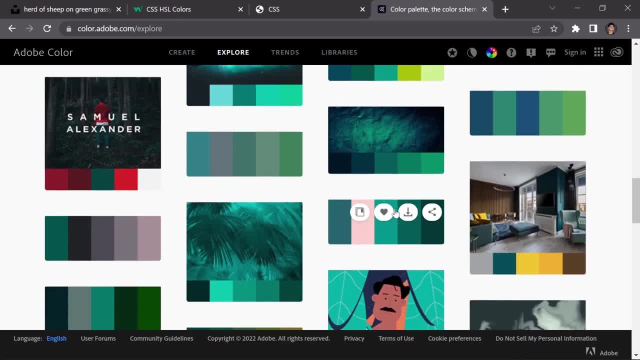 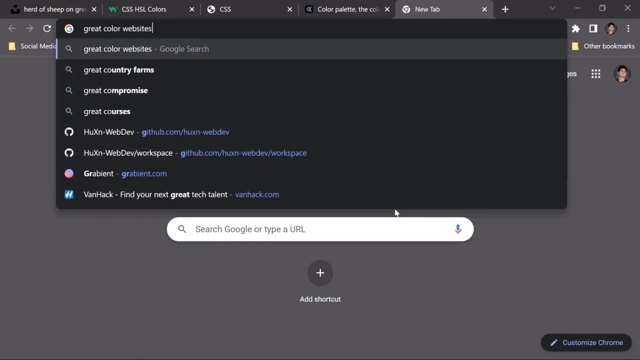 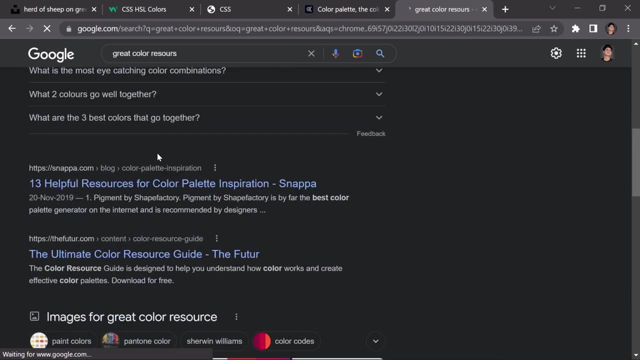 your library if you are working on that, or you can just get a color from there, or you can also just search for like: um great color, a website, um great resource, color resources would be fine- and then we have a lot of different kind of post. you know what. you can just go check that in your free time. but I guess I show you enough about. 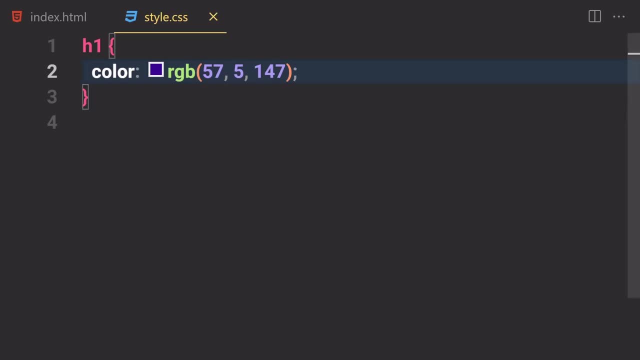 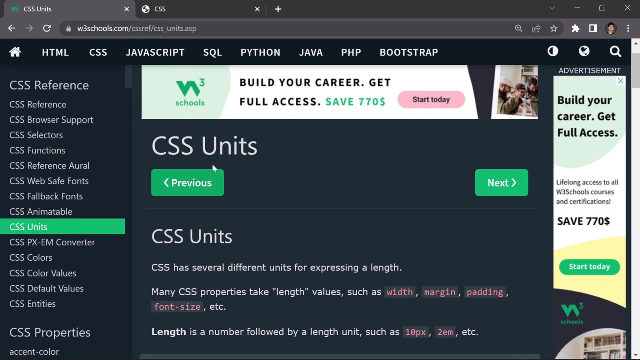 colors, and now you can go with your own direction with colors. all right, so now that we master colors in CSS, so now the next topic I want to share is something called CSS units. so if you ask our good, so here you can see. I'm now inside the CSS units page right here, and you can learn more about that. 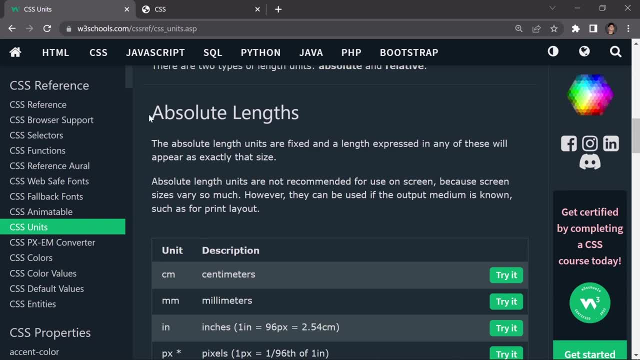 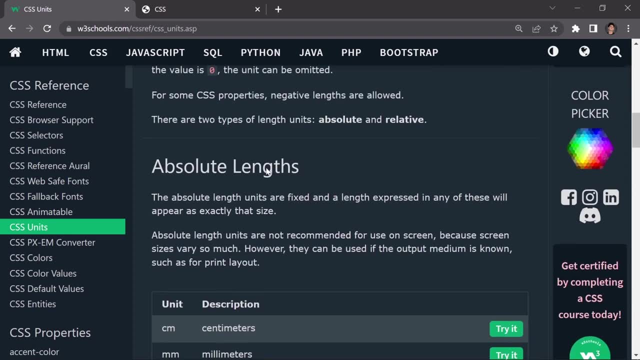 if you want to, but in my case I'm going to just highlight two things. so the first units we have is like absolute lens, and then we have a relative lens. so what is the difference between both of them? so I'm going to just zoom in a bit so you guys can see everything a bit better, and I'm 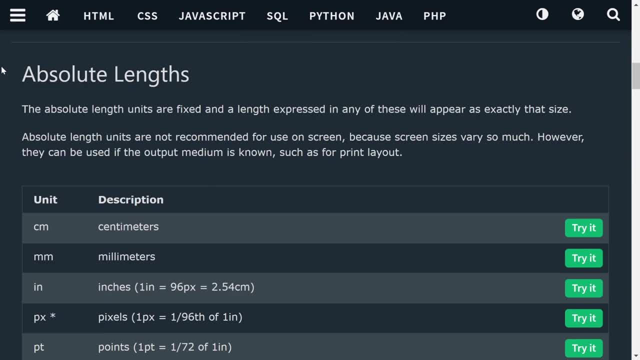 going to just head back over to that presentation mode right here. so what is the absolute lens? the absolute lens units are fixed and the length Express in any of these will appear as exactly that size. so you just have to remember that will be the exactly that size. okay, if you want to work. 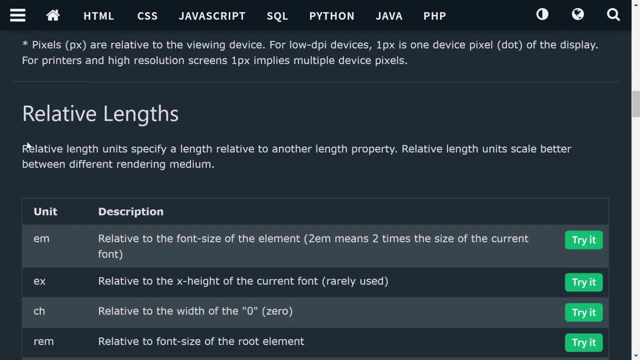 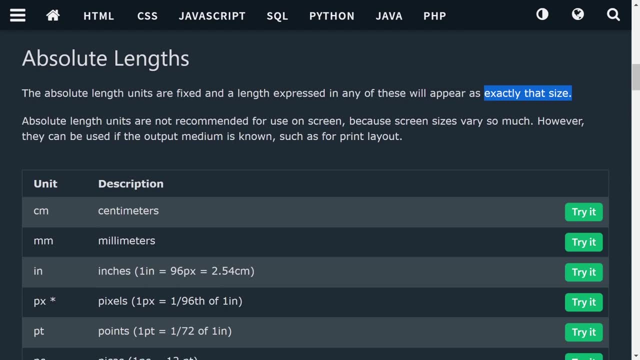 with absolute units. on the other hand, we have a relative lens, so a relative unit specify a length relative to another length property. okay, so this one will be the exact one, like exactly the size, and this will specify to the another length property, and so you just have to remember the. 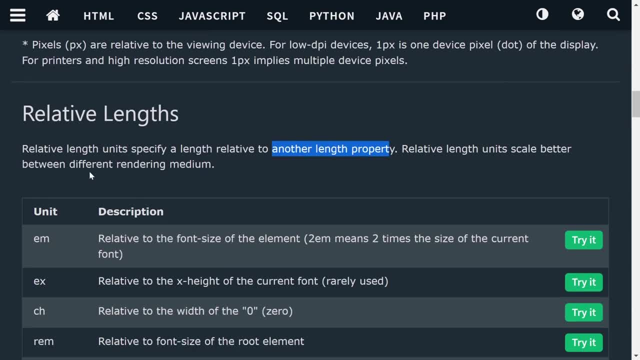 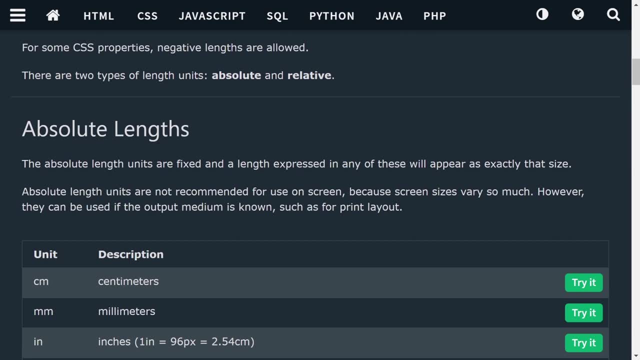 difference between both of them. okay, and relative lens units scale better between different rendering the medium and in this case they say: like absolute lens units are not recommended for the screen because screen sizes varies so much. however, they can be used if the output medium is known, such as: 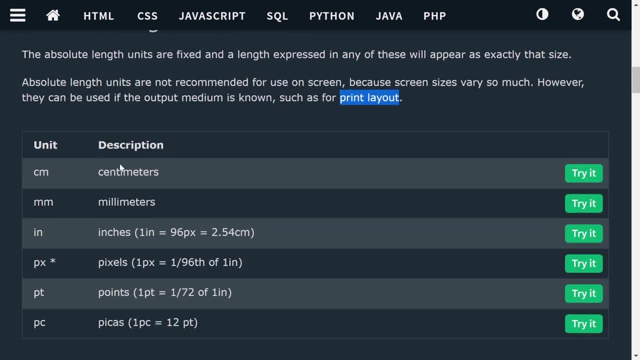 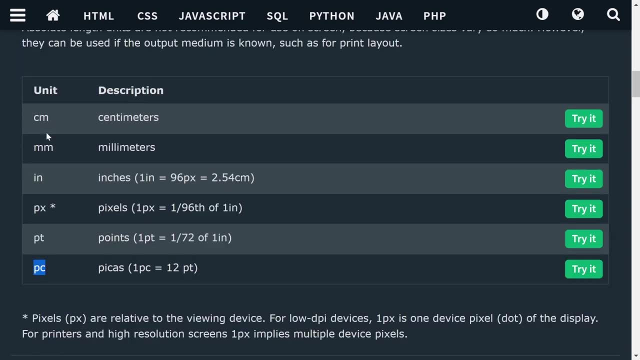 for, like, print layouts and stuff. okay, so we have first units. first of all, so we have CM MM in PX, PT and PC. to be honest, you would never use any of them, but you will use this PX and this is known as a pixel, and pixel will be just like a dot in your screen. okay, so if you want to get more into, 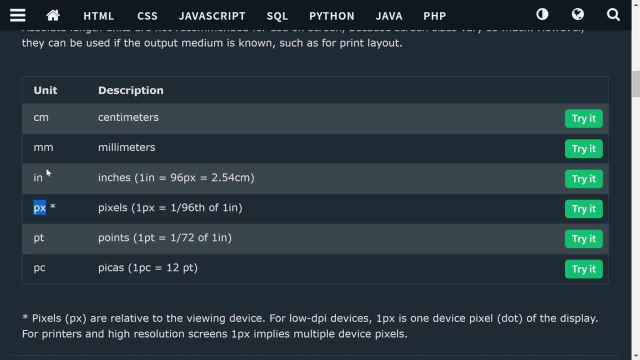 detail of that. you can just click Google search like what is a pixel, and you can learn more about that. okay, so you will never use like CM. I shouldn't have to say never, but you will never see this CM use in some CSS properties. okay, so we have a CM which stands for like centimeter, then we have MM for millimeter, then we have 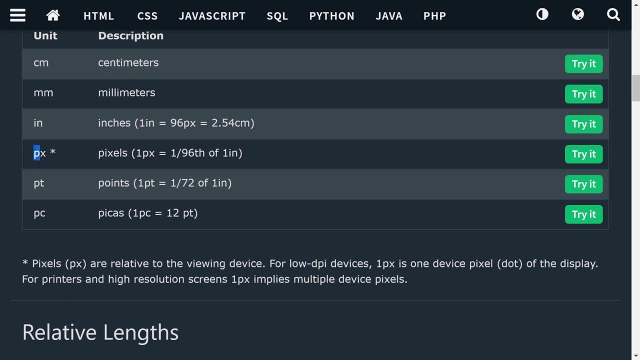 IN for inches. then we have a PX for pixel, a very widely used like a pixel unit. then we have a PT for points and then we have a PC. I've never in my life even see this one for sure. we all know what I used sometimes we. this is p, conv or pack. I can't pronounce you in the name. 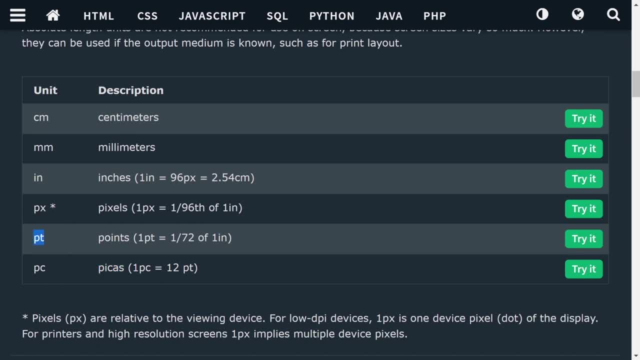 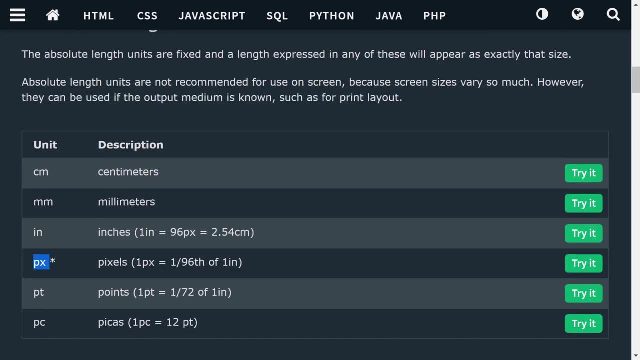 of it. so in this list, we are just interested in this one. uh, not this one. this one right here, pixel. okay, so you can learn more about that, okay, but before we learn about that, first of all we have to write some codes. so what I'm going to do is that I'm going to remove this H1 from here. 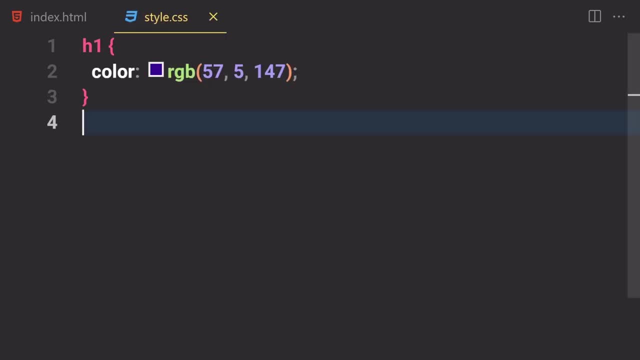 and I'm going to just declare our div right here. I'm going to save that file, I'm going to also remove this H1 and I'm going to write my div and I'm going to give a width of like in this. if you want to provide a width to something like it, doesn't matter like you want to provide for. 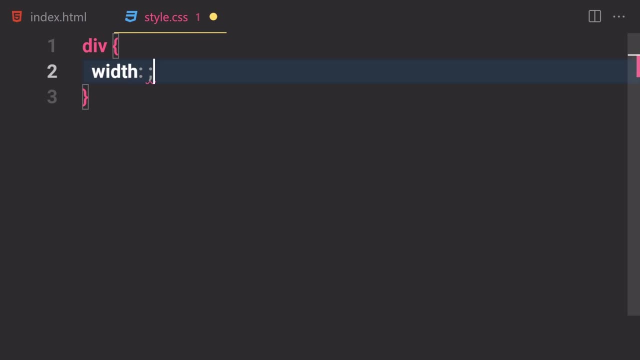 h1 header, section navigation, whatever. so if you want to provide a width to it, so for that we are going to be writing a width property, okay, and then we can specify the amount right here, okay. so in this case, let's suppose, if you want to provide like 100 pixel, so here you can see, we 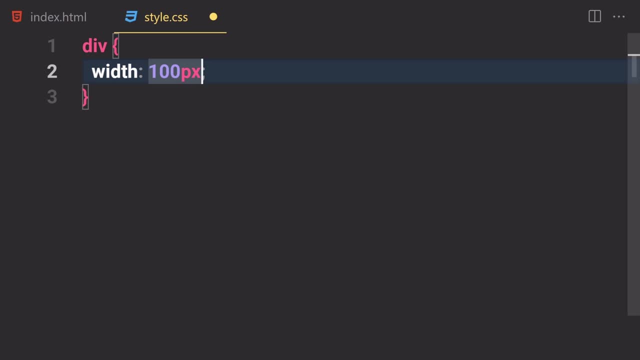 now use this px and fun log uses like 100 dots on the screen. okay, then we have a height. if you want to specify a height for something, so for that we can use, like this height property and then specify the amount of height you need. okay, so now, if you save this file and if you go to or 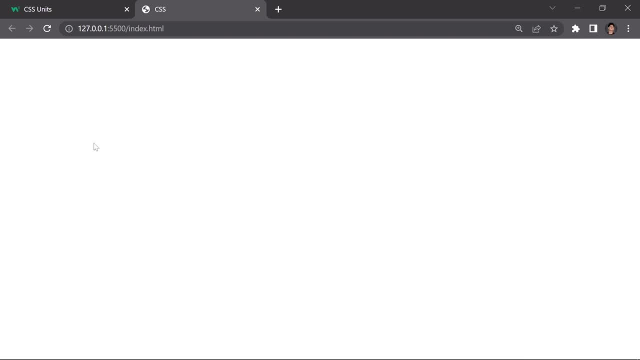 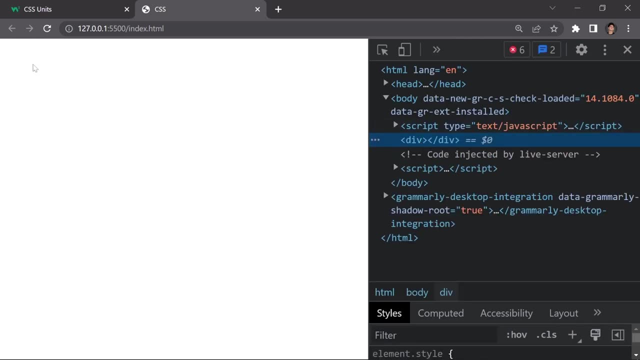 file right here. so what do we get? we get nothing right here. what div is right here? if you right click on it and click on the inspect. so here you can see we have that div. and here you can also see, if i hover my mouse over here, you can also see that blue area which is highlighting this div. 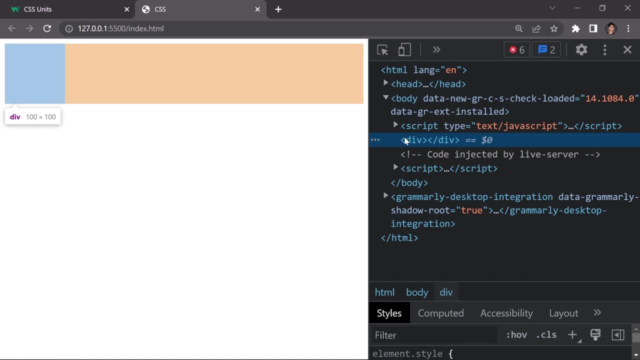 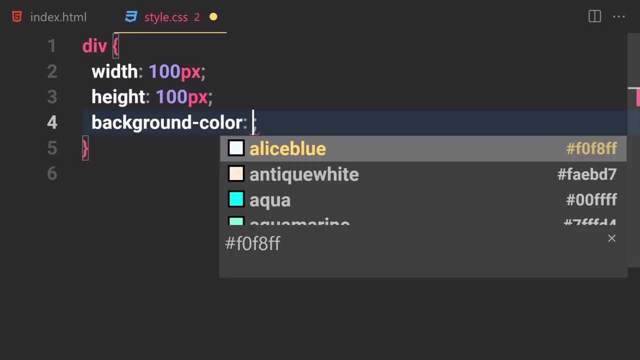 but we don't have any content and we don't have any like like border and stuff, and you don't have to worry about any of them, because we are going to be just writing like a background and then color, which we learned just a second ago and we can just provide. 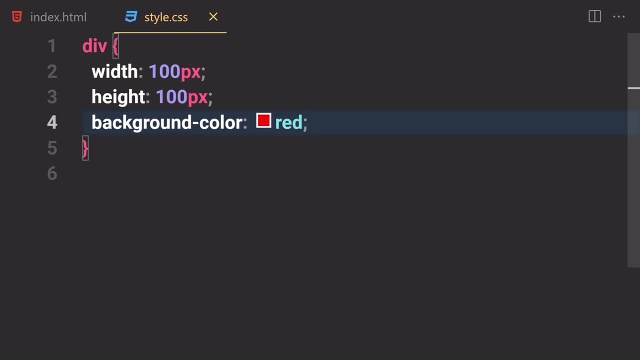 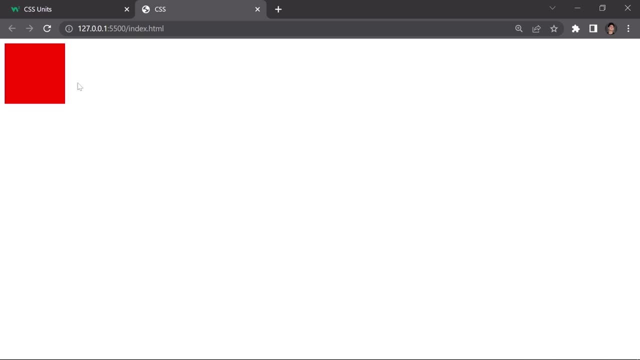 what color like in my case, i'm going to just write red. and now if you save file and boom, here you can see we have our div right here, which is 200 by 200. okay, so it will now give us like 200 width and 200. 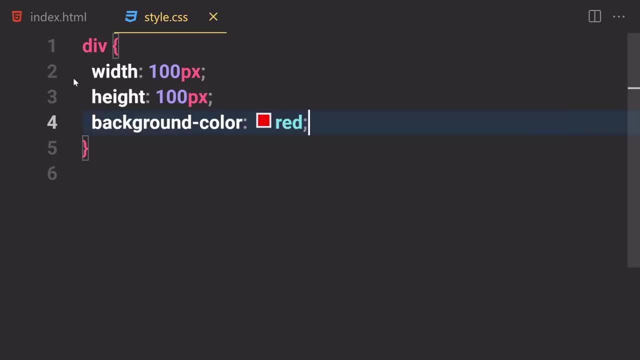 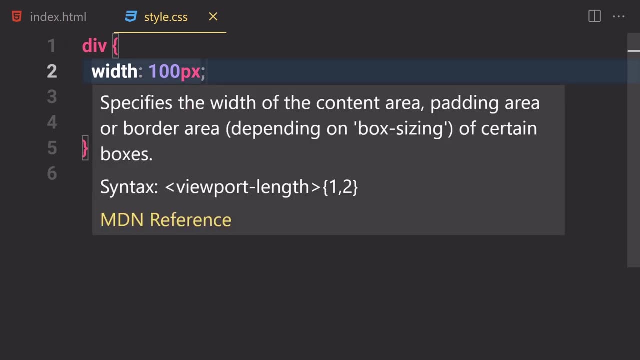 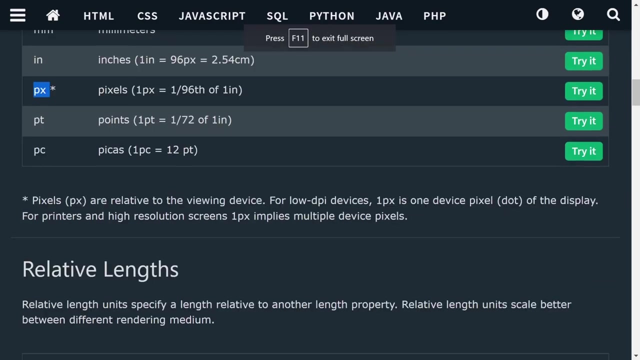 height. okay, so this is the first unit which we learned in this section. so we have like 100 px, and px is 10 for pixel, and here you also saw that these are absolute units, like pixel is absolute unit of measurement. and then now let's learn about our relative units. so we have a lot of relative units, so we have m. 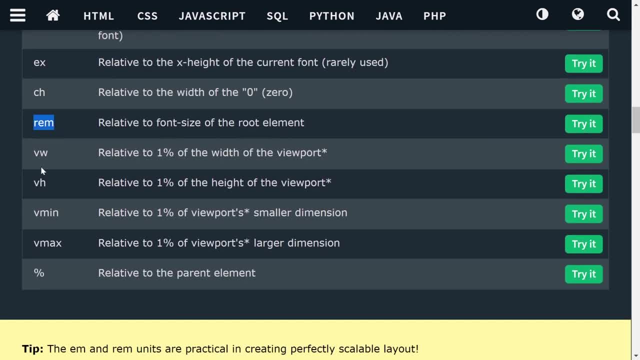 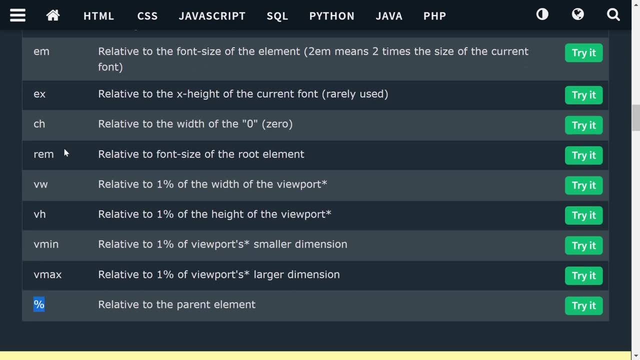 we are going to be learning about m and we are going to be learning about ram, vw, vh and, finally, percentages. okay, you can learn more about the other one. i have seen them in some projects, but i have never used it. i shouldn't have to say never. i did use that in some cases, but but not that often. 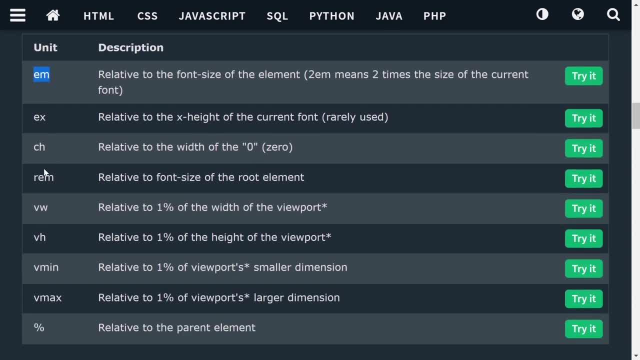 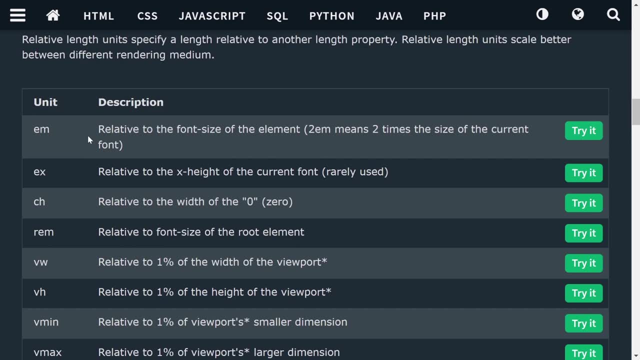 so i'm going to show you how to use it in some cases, but i'm going to show you how to use it in. just highlight these few. so we are going to be learning about m. we are going to be learning about rem, vw, vh and percentages. okay, so, starting from the first one, uh, which will be a percentage. so 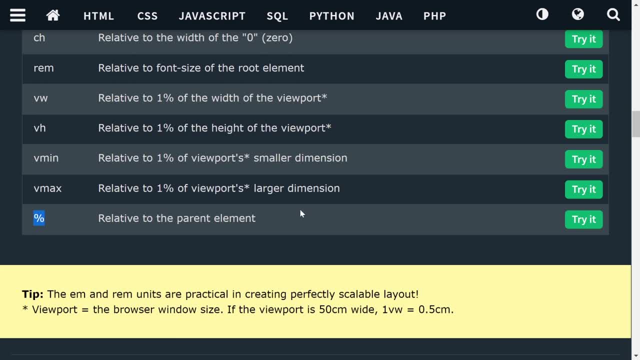 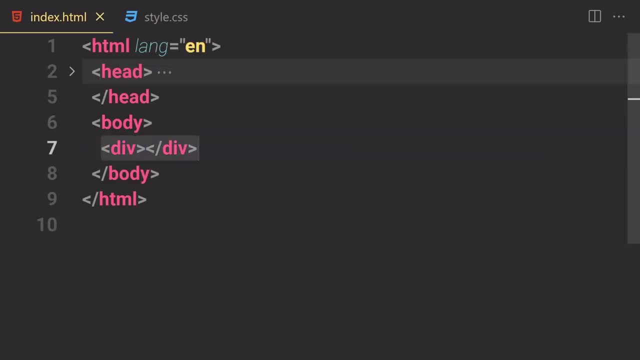 a percentage is the relative to its parent. so now let me just write some code, then you will get to know what i'm talking about. so, now that you can see, we have this div right here. so what will be the parent of this div? the parent will be this body right here. so what will be the parent of? 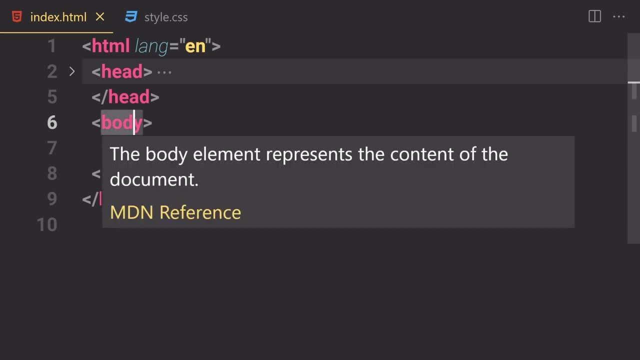 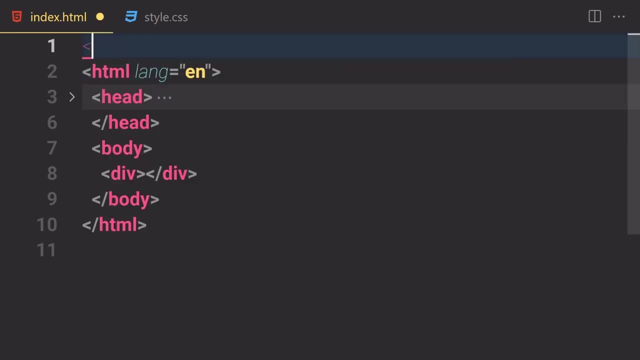 this body. you might be guessing like it's a head, but it's not a head. the parent of the body is this html. okay, so what is the parent of this html? i forgot to include a doc type in here. uh, okay, let me just write it doc. oh, my goodness, doc type and then html. and now let me just close it right here. 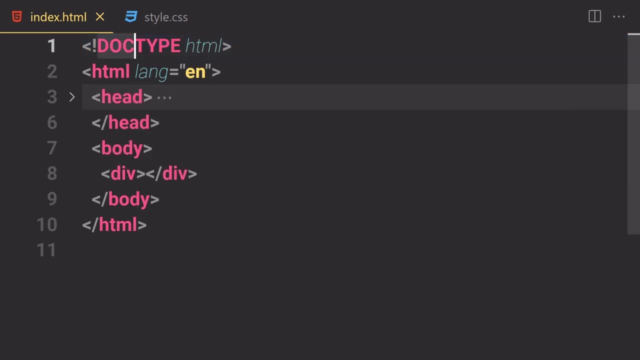 okay, so the parent of this html will be this doc type. okay, so now, if you want to wrap that in some sort of a parent, so for that we can use like a section or article or whatever. you want to wrap that in some sort of a parent, so for that we can use like a section or article. 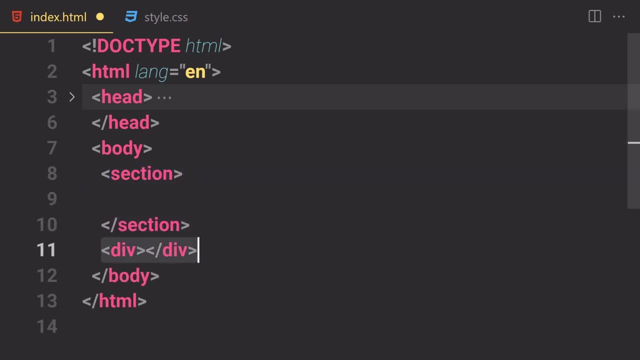 you have. so now, if i hit enter right here and now i'm going to cut this uh div from here and i'm going to paste it right here. so now the parent of this div is now a section, so this will be the parent and this div will be the children. okay, so now let's suppose, if i just write something, 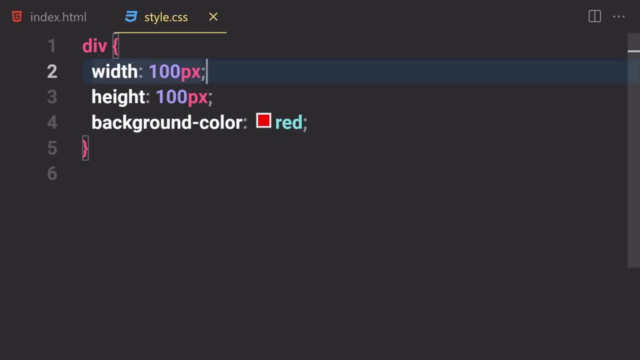 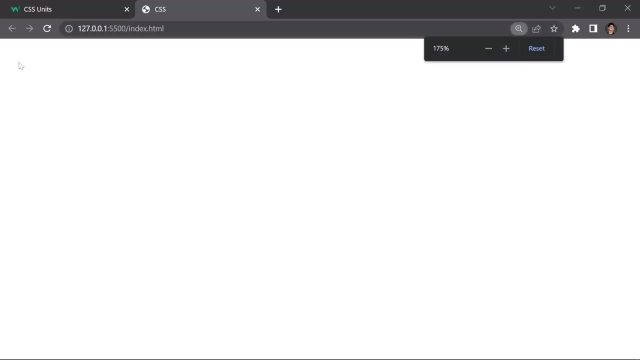 by using or parent. so instead of these pixels, if i just remove there and if i just write like a percentage right here and also percentage right here- and remember we didn't write any styling and whatsoever for this section- okay, so now if you save a file and here you can see nothing is up here. okay, like this is totally empty. 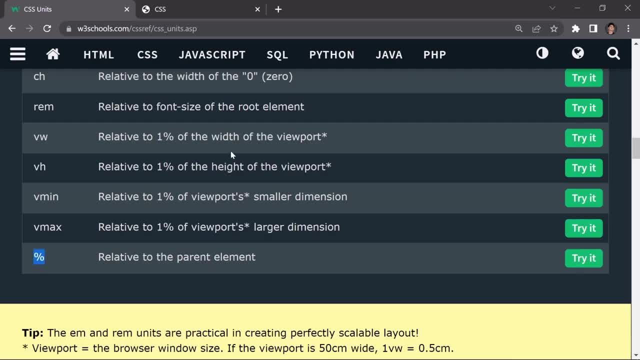 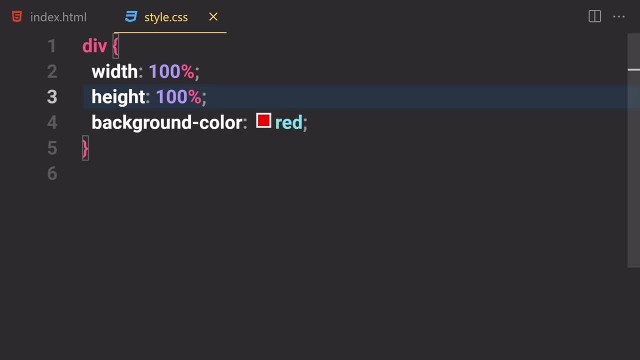 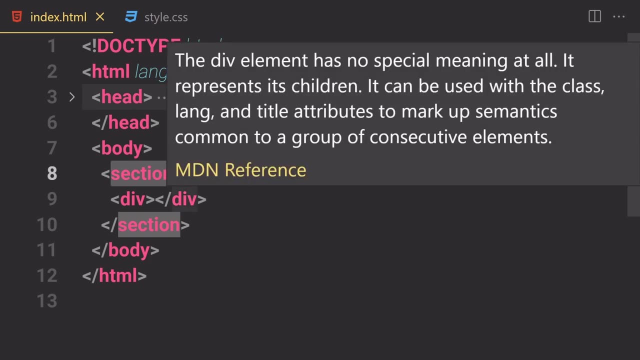 we cannot see anything why? because, as we learn right here, that relative- uh, i mean like percentage- is a relative to the its parent element. so we don't have any width and height to the parent element, so we don't specify any width or height to this section. so that's why we cannot see nothing. 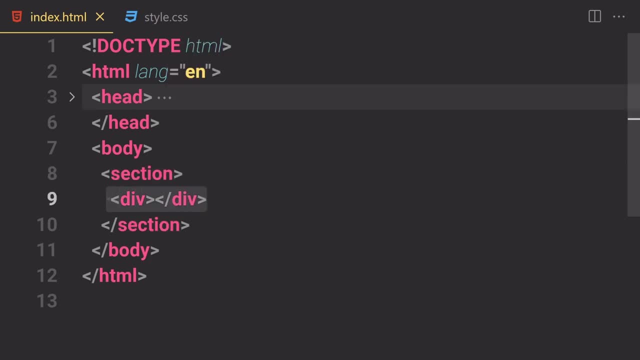 okay, and we are specifying a hundred percent width and hundred percent height to this div, but we're not sure because we don't have any width and height on this section. okay, so if you want to work with this section, first of all we have to select our section. so i'm going to just write a section right here. 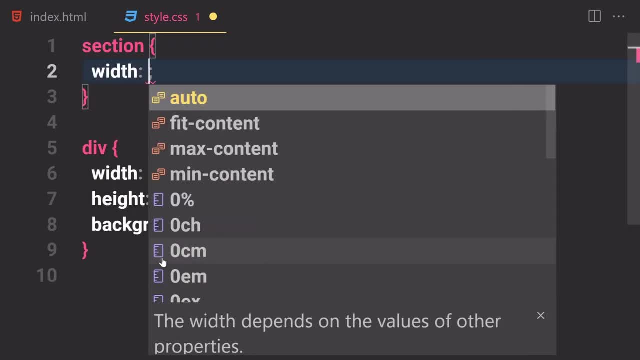 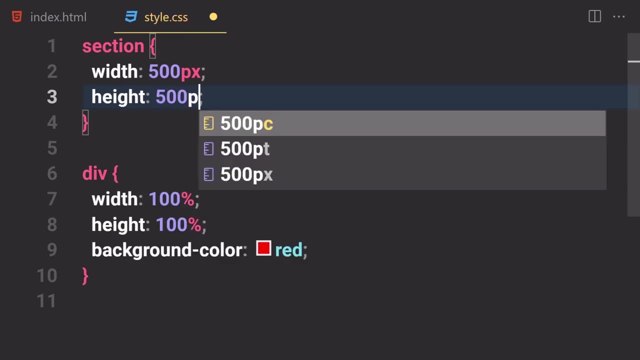 and inside there i'm going to just write a width of like- uh, i don't know- 100, not 100 pixel, but you know, i'm going to write like a 500 pixel and i'm going to also write a height of 500 pixels. so if 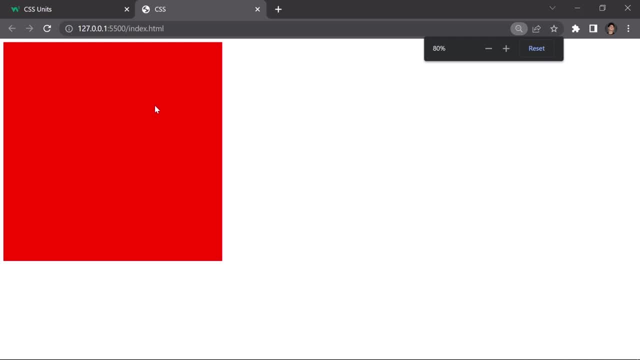 you save that. and now, here you can see, we get this huge box right here, so we have like 500 by 500 box and now the color is totally red right here. so we're going to just write a width of like a 100 and also the width we got here. we can just write the width of this section, we can just write. 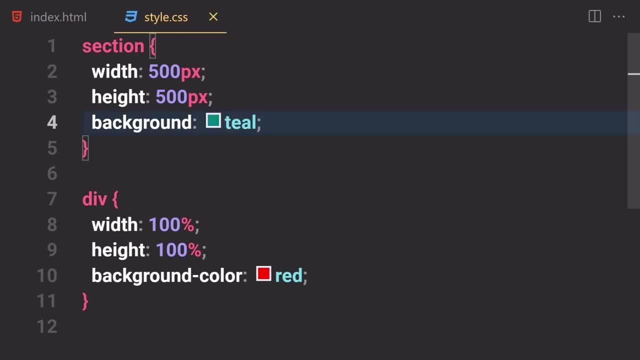 like you know, 100 and 100 pixel in this section. you just have to type this kinda figure right there and that's how we're going to do this. okay, so why is the color totally red? let's suppose if you just provide, like the background color to be like teal, maybe so if you save our file, and why is not that? 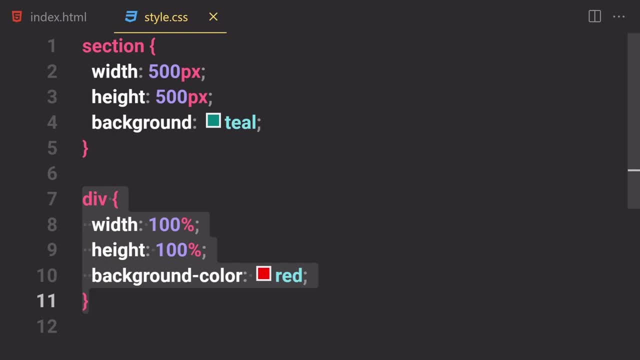 teal showing up right here. that's because this div is now the children of this section and we are providing 100 of width to it and 100 percent of height to it. so now this div is tagging all of the and now, if you save that- and now here you can see- it will now just take the half of this div right. 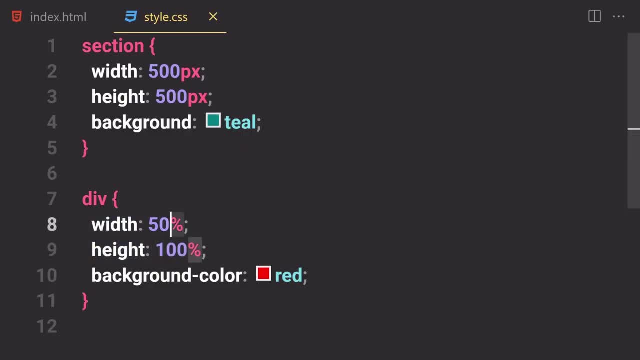 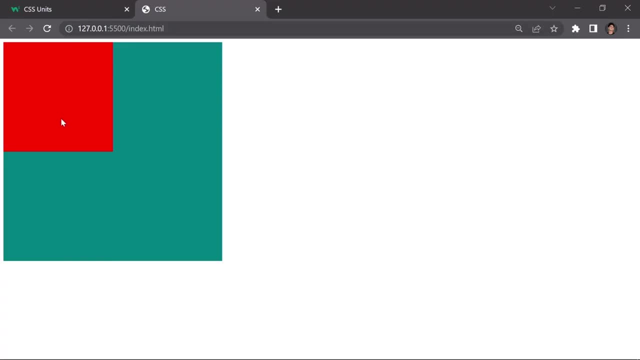 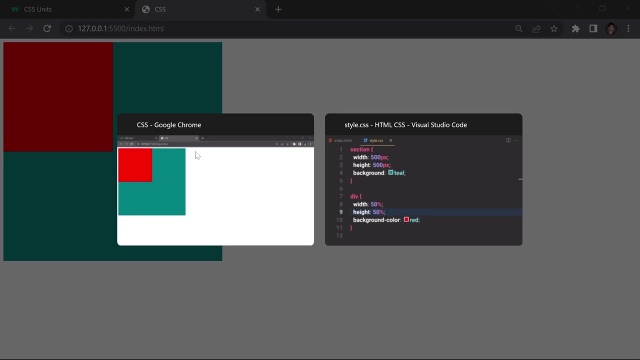 here half of the section area, because we are now working on percentages right here. so now let me just write a height as well. so if you just write 50 of height and if you save that and now here you can see, this is now 50 by 50 and this one is 500 by 500. okay, so this is how we can work with. 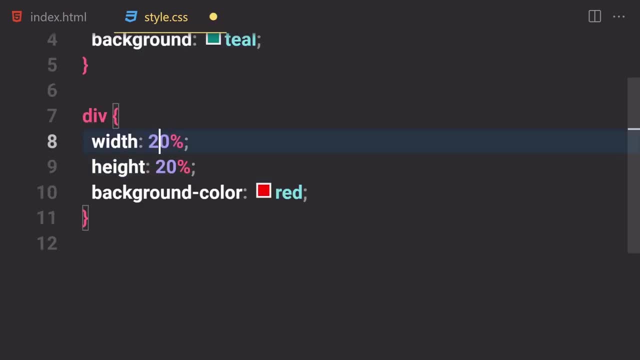 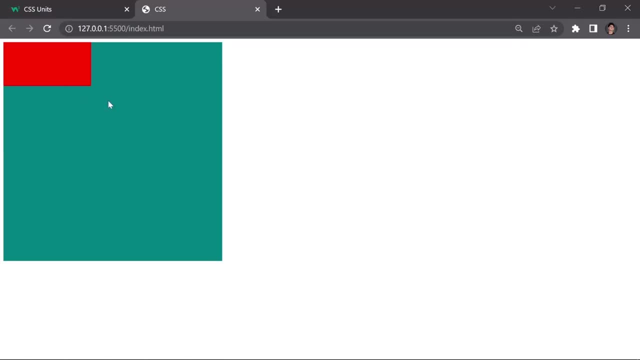 that. so let's suppose, if you just want to write like 20 and then 20, or you know 40 and 20, so this is how it will look like, and so on and so forth, so you can play around with that if you want to. 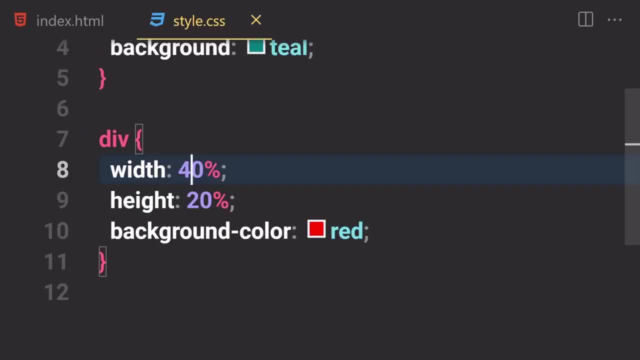 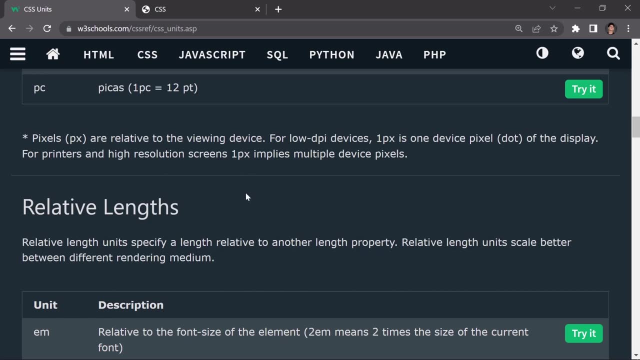 but we are totally done with all right. so now that we learned two units- so the first one was a pixel and then the second one is a percentage. so now let's just learn more about a relative unit. so the first one we have is an m, and m is a relative to the size of the font size. 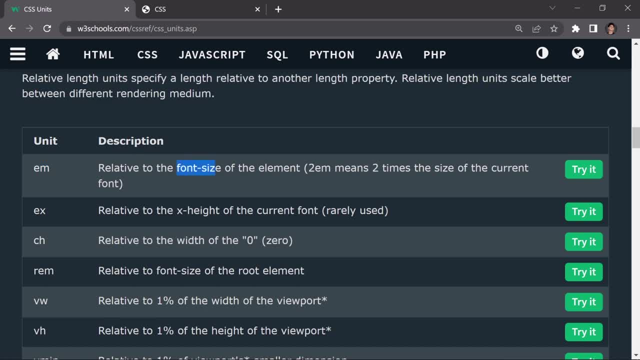 of the element. so, which means like 2m means two times of the font size of the current font. okay, so what is all of this gibberish means? so for that i'm going to remove everything. okay, so now let's just write a height of 20, and then we're going to write a height of 20. 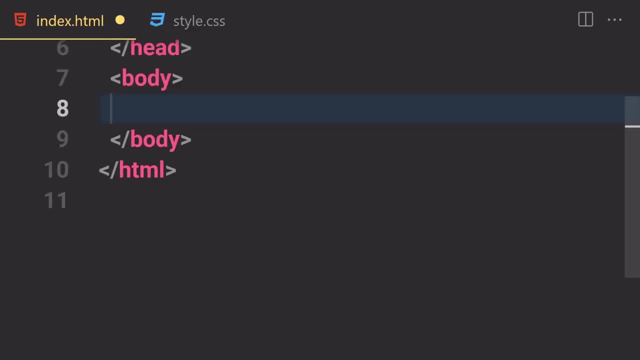 which i have inside a css, and i'm going to also remove this section and their dev. so we have now empty body, right here and now. what i will do is i'll just first of all select like html, like the root tag, and let me just save this html file and i'm going to just provide like a font size of. 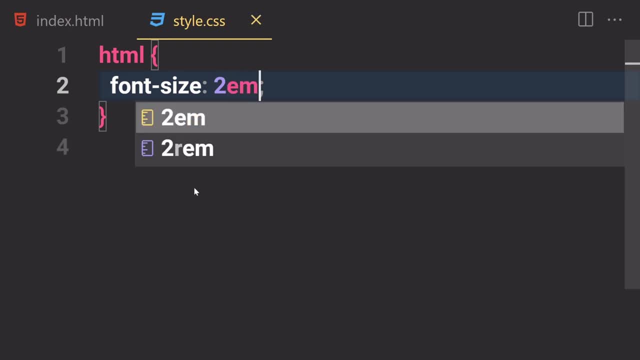 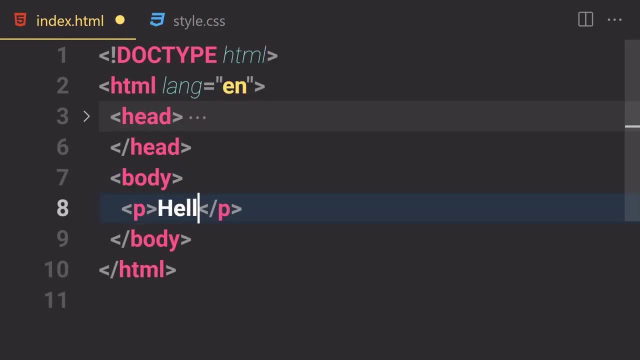 2m. okay, by default i'm going to just provide like 2m. if you save that and we cannot see something because we didn't write any text and whatnot. and now if you just write like uh, hello, inside this paragraph, and now if you save that, and now here you can see it when i'm 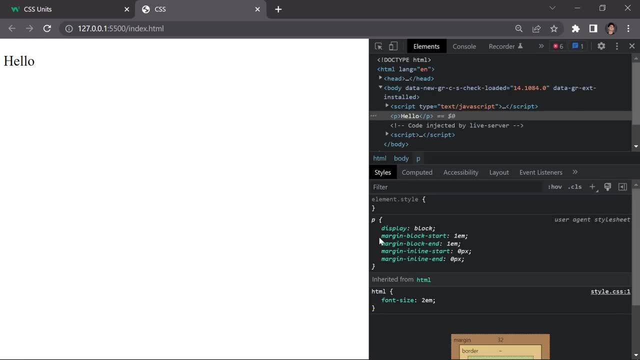 using like 2m, if you right click on it and click on inspect, and now, here you can see, it will not use like font size is 2m, but if we uncheck that, so here you can see, it will not use, just in 16. 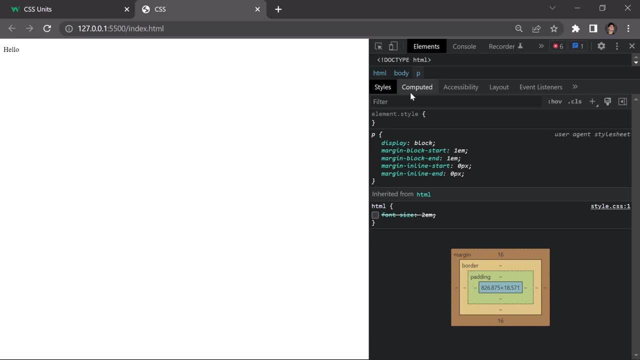 pixel and what is the default size? okay, so if you go to the computer values, so here you can see, by default the font size will be 16 pixel. okay, so if you just check that and we provide like 2m, so here you can see, it will now double the size and we have now 32 right here. okay so, 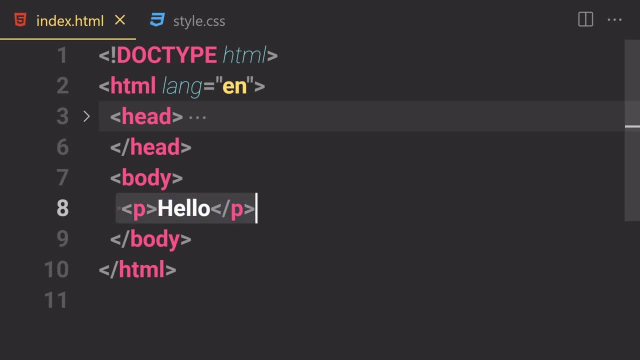 this is what's going to be happening, and we can also change this to like something else, like if i just go to my paragraph and, by the way, i forgot to show you like, font size is a property which allows us to increase or decrease the sizes of our font, and 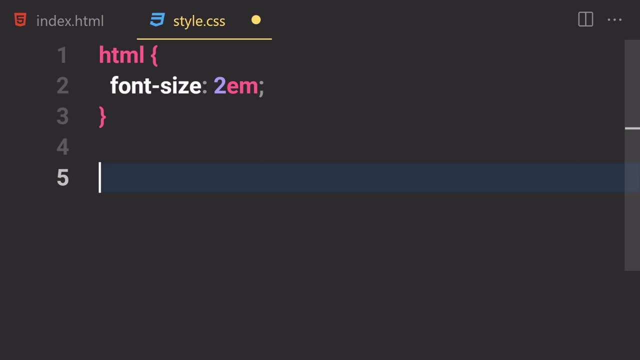 we are going to be diving into the font sizes and typography in a really great detail just in a second, but for now i just kind of want to show you everything like what is the m unit working and stuff like that. okay, so now let me just select my paragraph in here, and here i'm going to just 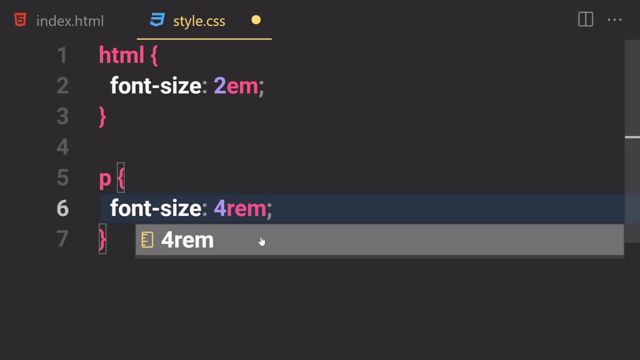 like a font size of maybe 4m right here. okay, so not rem, but m. so now, if you save a file and now here you can see, it will now bump it up. why is that? that's because we provide this font size of 4m right here, but if you comment this line out and if you save that and here you can, 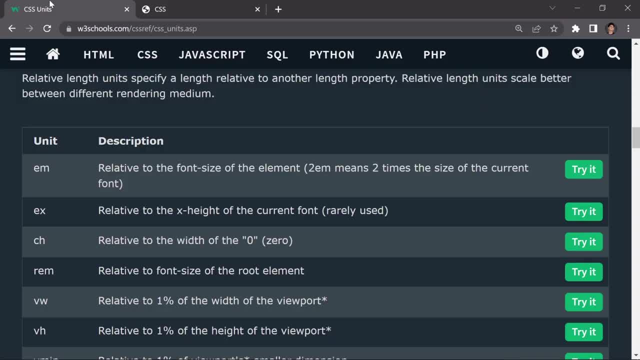 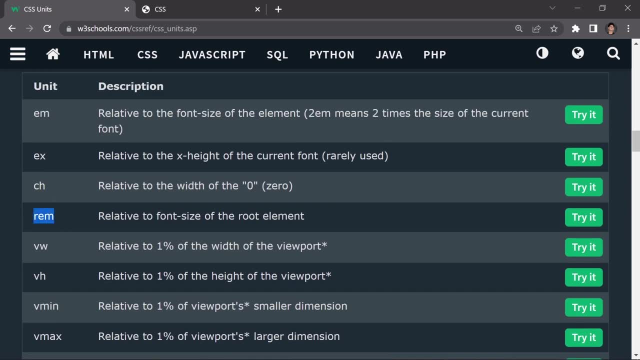 see it will now make it smaller right here. okay, so this is how we can work with the m unit. now let's learn about the third unit which you're going to be learning, or maybe the fourth one, which is a rem. so rem is relative to the font size of the root element, it doesn't care about. 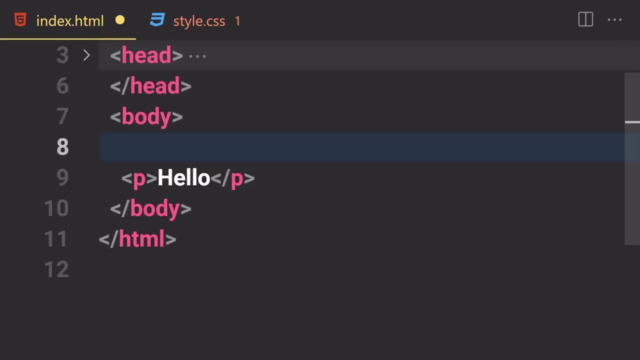 the parent element. like if i just write a parent element, if we have like parent element right here section, and then if we cut this paragraph from there and we put it right here, so this is now the parent element and this is now the children element right here. as i told you that in a second 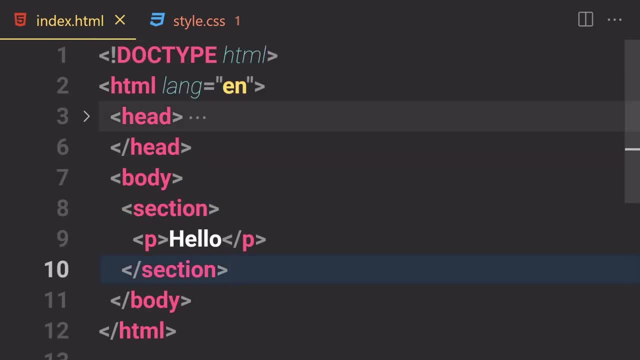 so now if you want to use a rem unit, so rem unit doesn't care about the parent element, if i'll just go straight up to the root element right here, so it will just check the font size. if the font size is something like maybe 16 pixel and we write like two rems, so it will now double up the font. 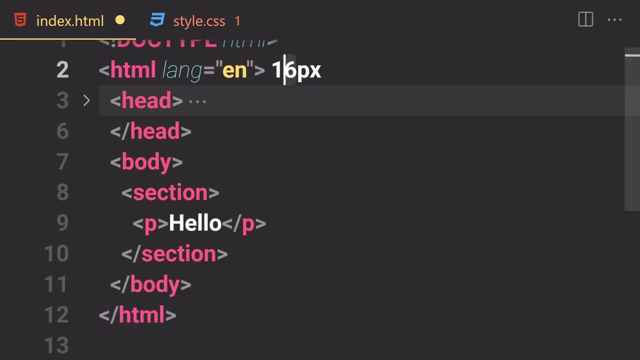 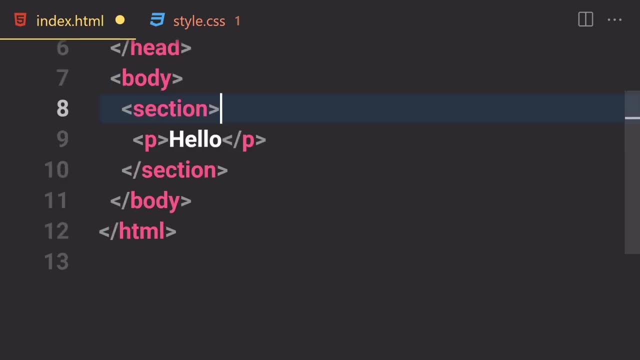 size to be like 32, so it will now change the font size to be just 32. okay, so let me just show you that in action and then you'll get to know what i'm talking about. so i'm going to remove this section from here and from here, and if we save, 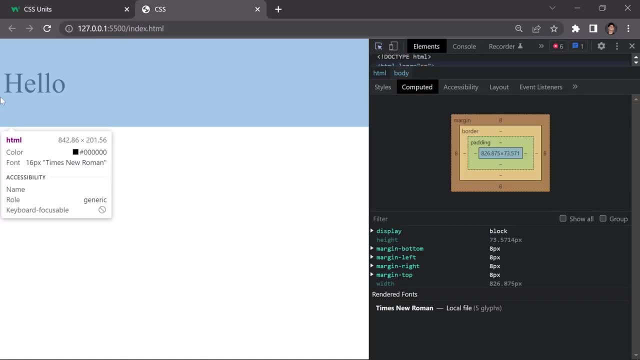 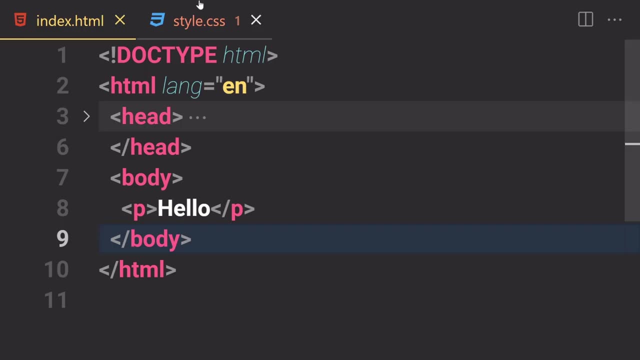 that and this is how everything currently looks like. and if you click on it and click on it one more time, so i want you to notice this font area, it is, by default, 64. what is going on? uh, okay, we provide this. i'm going to remove this from here and now. here, uh, their font family is gone because 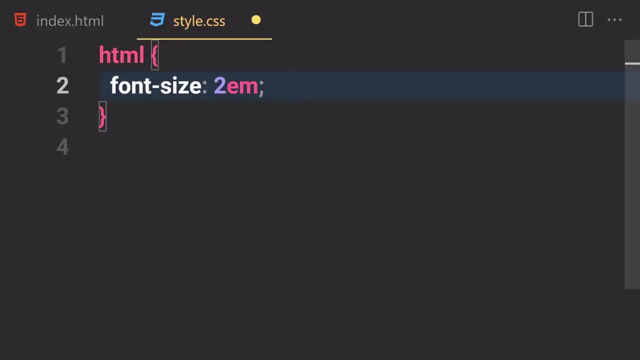 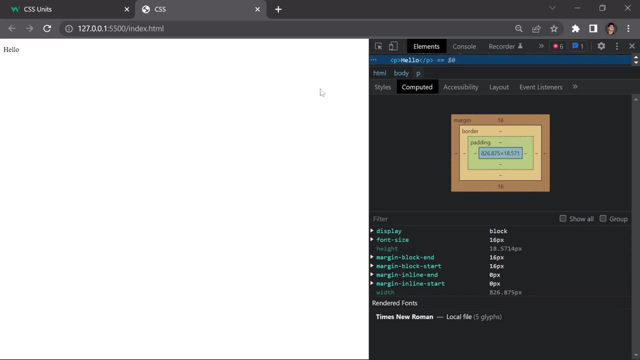 we're not providing a font family to it. but if you want to provide font family, so we can also do that. but let's suppose if i just write like a font, i'm going to write like font size of 16 pixel if i save my file. and now here you can see, we have a. 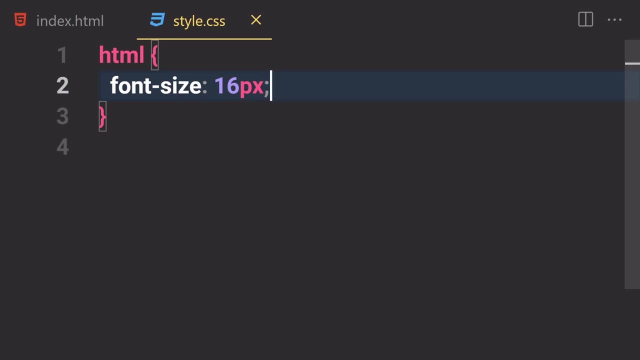 font size of 16 pixel right here, okay. and now, if you want to work with a rem unit, like, uh, if i want to change the font size of this to like two rem, so for that we can use like first of all paragraph and now i'm going to write like font size of two rem, okay, so if i do that, uh, so now let me just 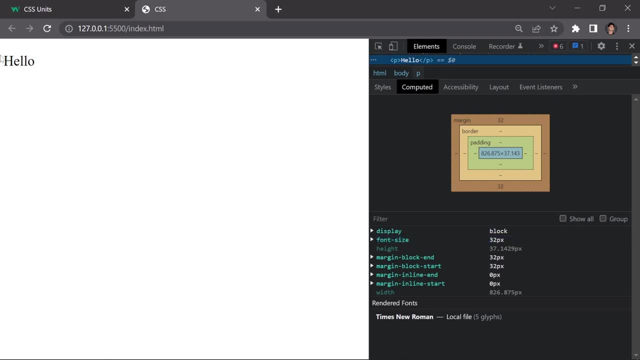 save my file. and now here you can see it will now double up that root element, a font size right here. so back then it was just 16 pixel, now it's 32 right here. but and, by the way, one rem is equal to 16 pixel. so if i just write like one rem and if it's several, 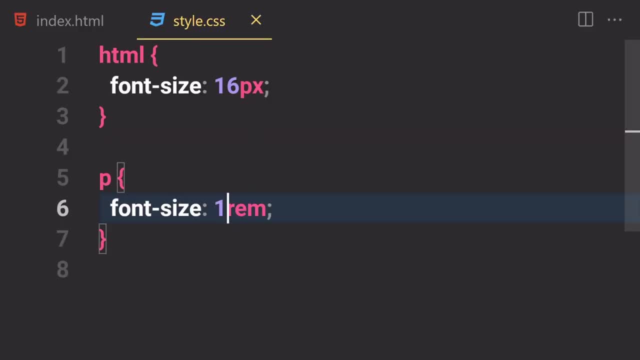 file, it will be just 16 pixel. and if you just write like two rem, so then we have 32 rem. if you write like uh, three rem, so here you can see the log is 48 rem. four rem will be just like 64 rem, i mean like 64 pixel. and if you just write five pixel, uh. 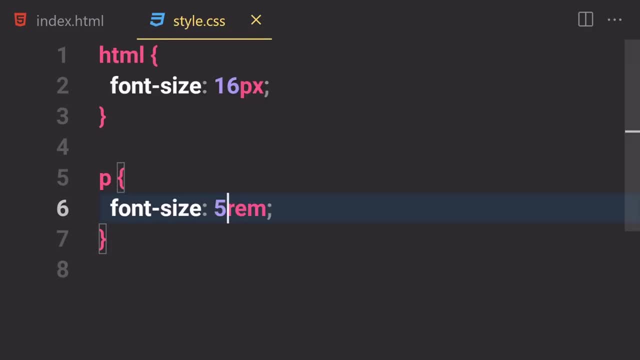 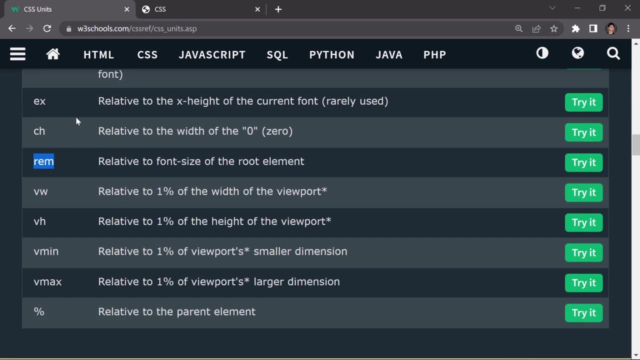 five frame, so it will be 80, so it can go on and on like that. okay, you can learn more about that if you want to, but i'll not suggest you to learn more about that. but you have to remember like we have these uh relative units inside a css relative and um absolute unit. so then now the 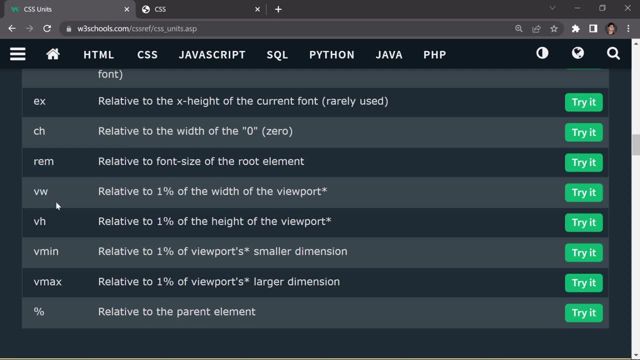 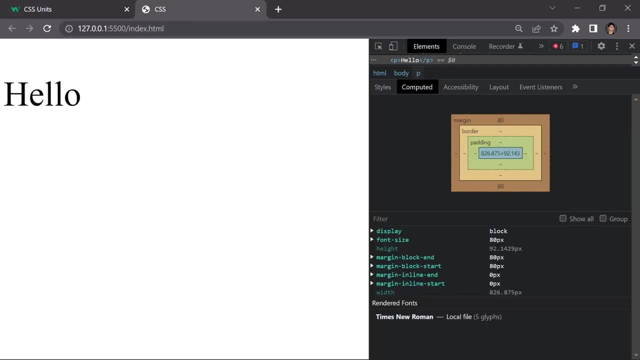 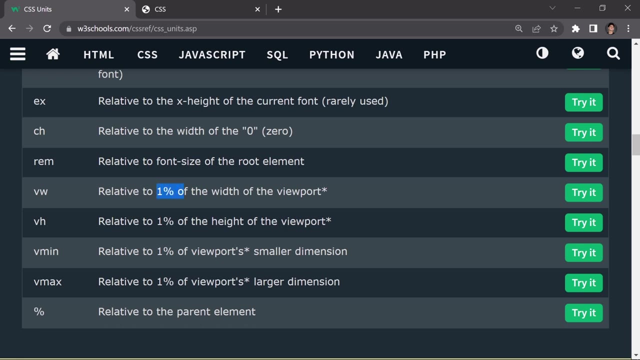 next one we have is this: vw and vh right here. so first of all, let's learn about a vw. so vw just simply means the viewport width. so what is a viewport? a viewport is all of this body area. so what is that saying? so vw is relative to one person of the width of the viewport, right here. 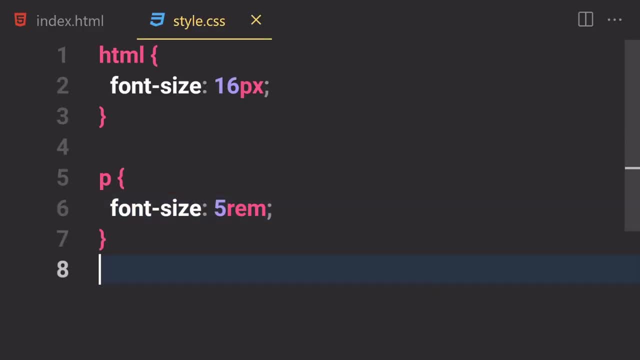 okay, so we'll just take one person of width if you just write like one pixel and stuff. so i'm going to remove everything from here and i'm going to just remove that from here. instead i'm going to write dev and now, if you save that and if you just write div and we provide a little bit of 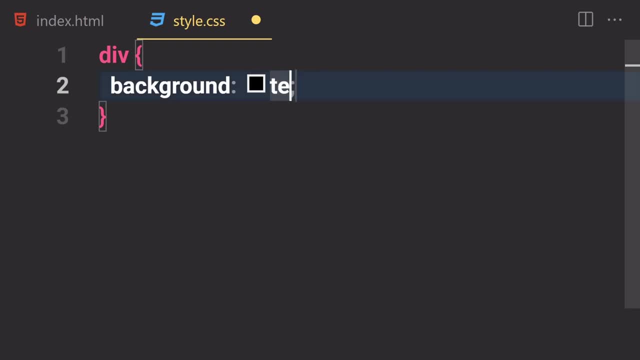 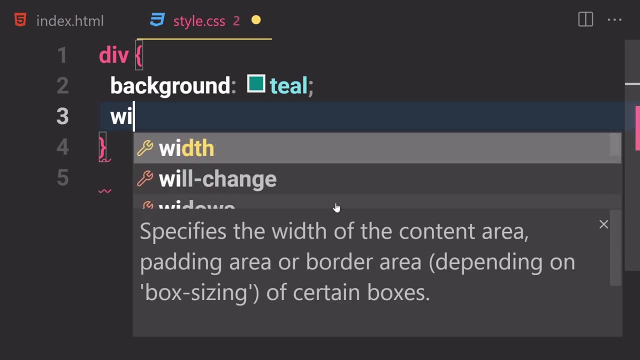 not width, but let me just write a background color of black or not black, but teal will be fine. if you save that, we cannot see nothing. so now, if you want to provide a width rate to it, so for that we can use like width property, as you saw just a second ago, you can give them. 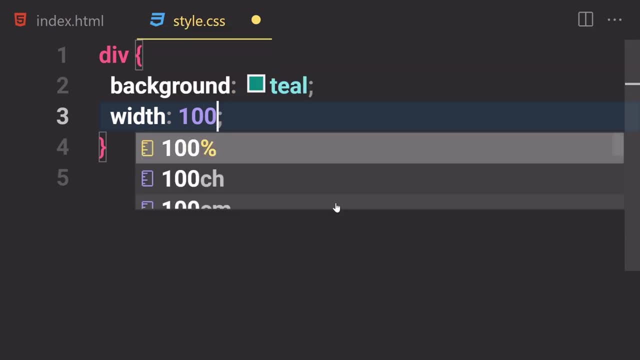 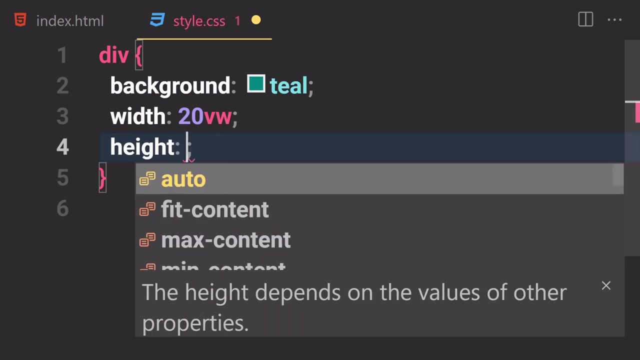 like 100 pixel or 100 if you want to. but in this case what do we have to do? we have to just write like 20 vw. it means that it will just take that 20 percent of the viewport width. so if you save that- and now here you cannot see that we have to provide height as well. so if you just write height, 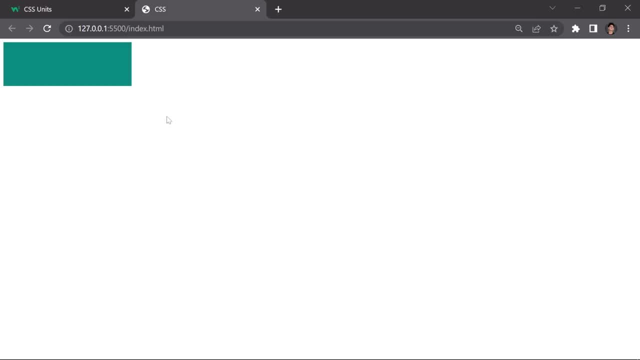 of like maybe 10 or 100 pixel if you save that. so now here you can see, it will not take like 20 percent of the viewport width right here. okay, if you want to take like 50 percent, so you can just write 50, it will now take 50 percent of the viewport width, and if you want to provide 100, so 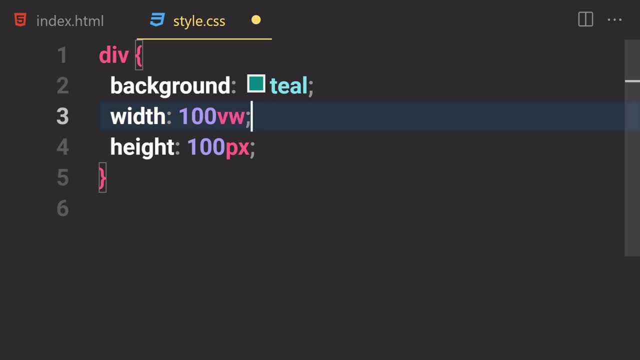 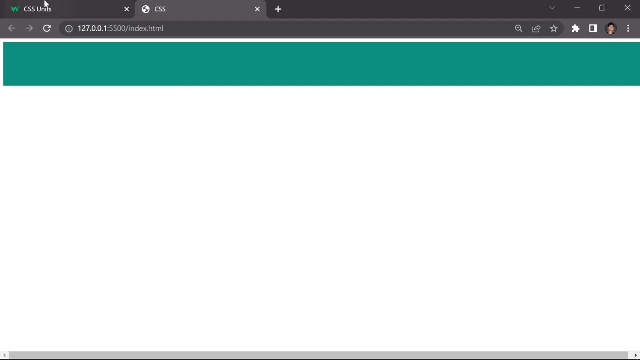 you can also write 100. okay, not 1000, but just 100. if you save our file and boom, it will take the entire width right here. okay, so the entire viewport width. and now the next one we have is a vh. so this one is a viewport width and this one is a viewport height. and now, if you want to change, like the, 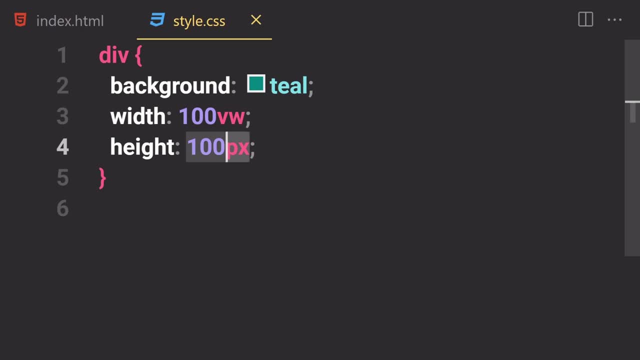 viewport height, so for that we have to just remove the viewport width. and now if you want to change like the viewport height, so for that we have to that pixel, and now we have to convert that to vh. so if you save our file and here you can see it. 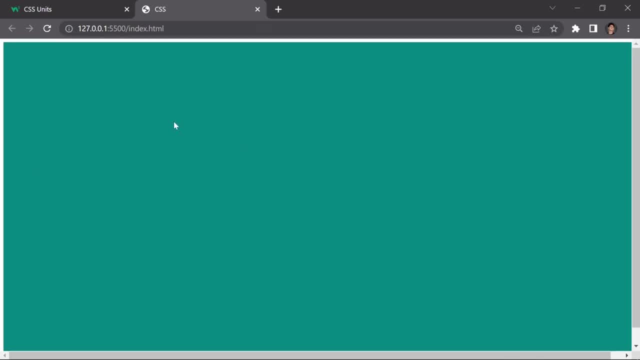 will now take the entire viewport right here. and, by the way, if you are wondering, like, where is this empty space is coming from, this is coming from something called a user agent style shield by the browser, but you don't have to worry about it for now, because we can remove that by using. 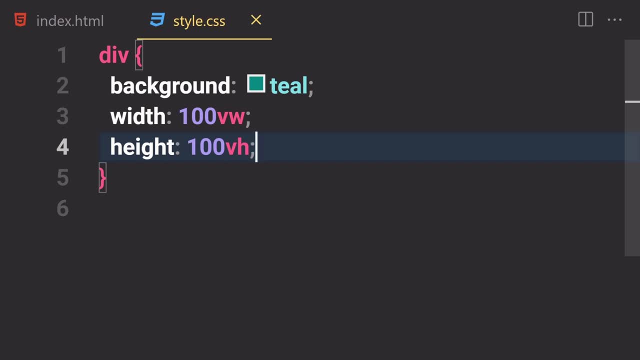 margins anyways. so this is it about a viewport width and viewport height, rems, ms, percentages and so on and so forth, okay. so if you just want to remove that viewport width and viewport height, rems, percentages and so on and so forth, okay. so if you just want to remove that viewport width and viewport height, 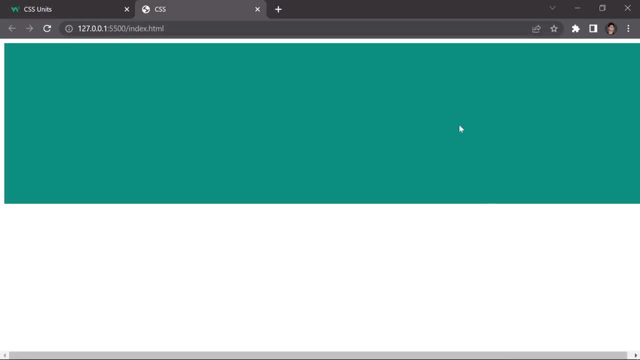 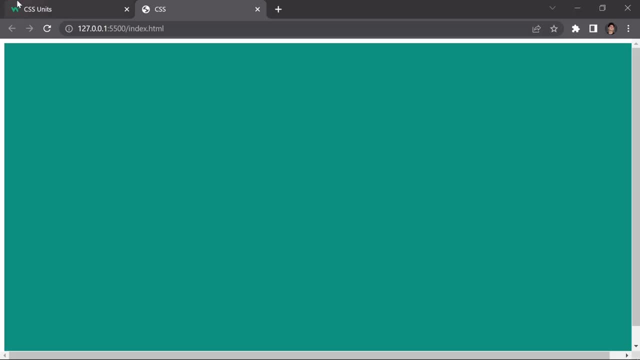 provide like uh, 50 percent of viewport height. so if you save that, so now just take like 100 percent of viewport height right here, okay, so we can play around with that if you want to, so you can learn more about that, and or you can just ask from google or you can go to the mdn if you want to. 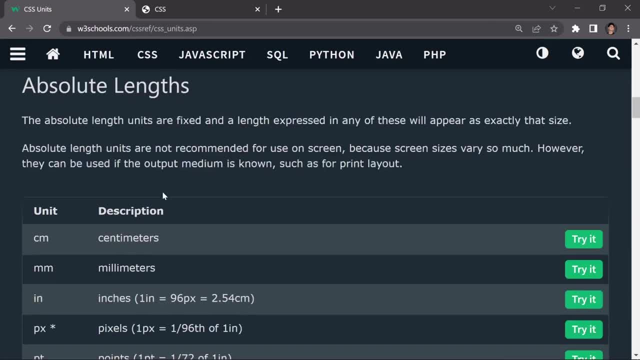 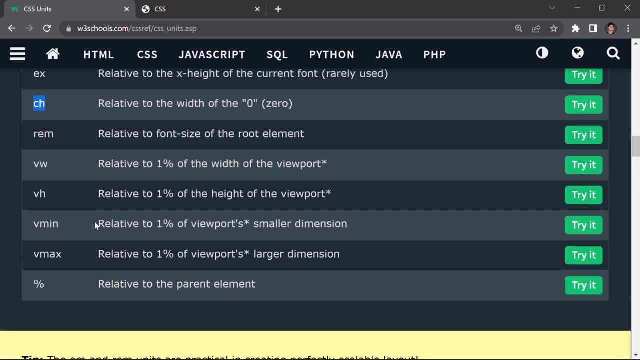 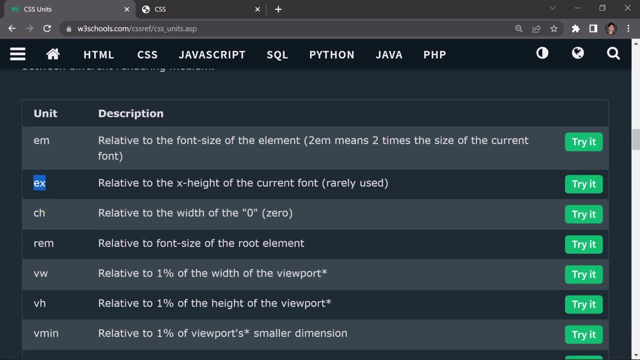 but my recommendation will be to not waste a lot of your time on a unit, so you can just choose one unit- and i have already mentioned all of them, except like ex and ch, and you would never use that in your life- ever. i shouldn't have to say ever. but you will use that, but you will not find yourself. 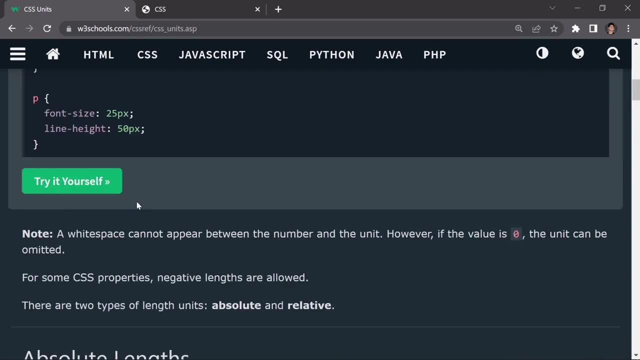 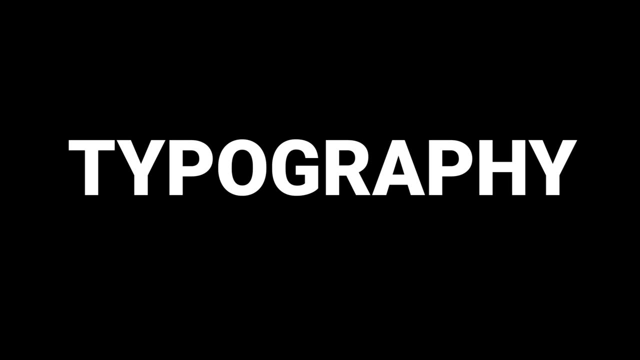 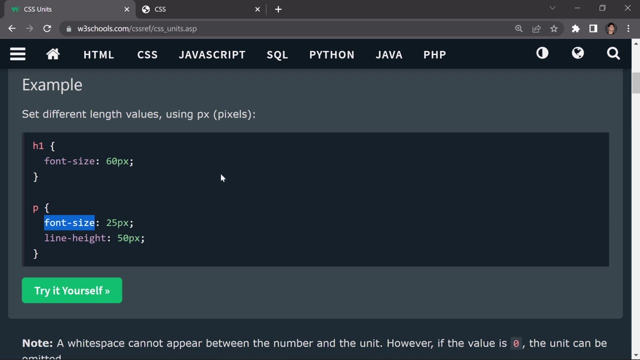 using all of them that much often, so i don't want to waste your time by explaining every single one of them. but now that you know units in css, all right. so i just show you a font size property, and this is a typography property in css. so what? 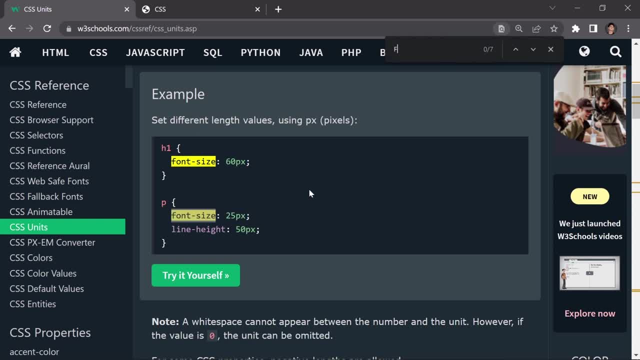 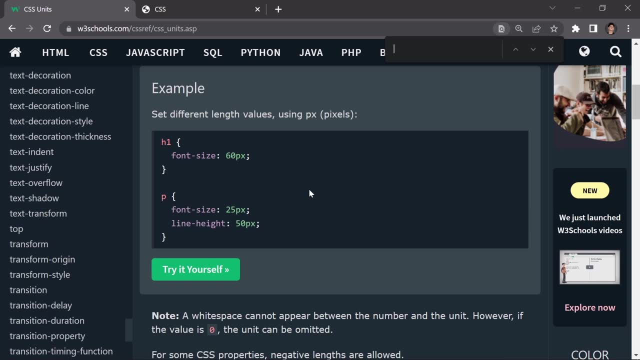 is a typography. if you just hit ctrl c and if you just write like formatting, okay, it's not helping me, f-o-r-m-a-t-t-i-n-g- okay, it's not still helping us. so if you just write type pography, okay, so it's not still, uh, helping us. if you write a font, okay. so now we have a lot. 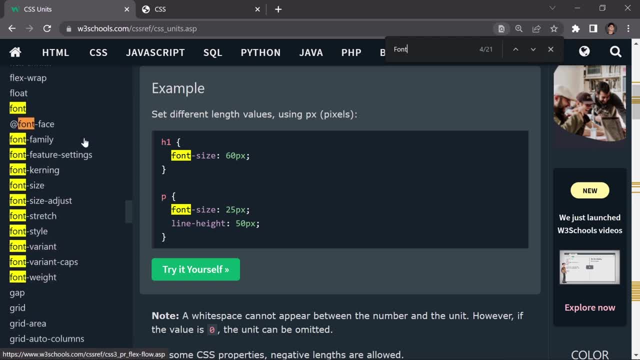 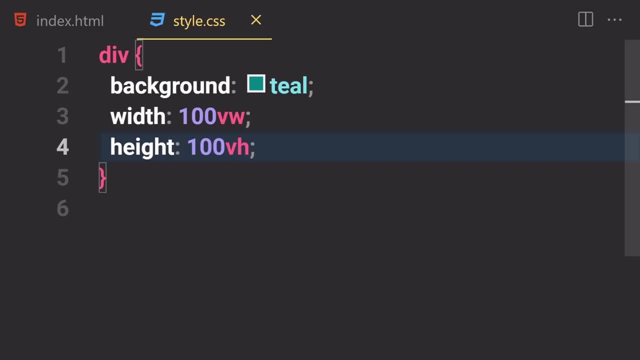 of kind of fonts and stuff. we have 20s- oh my goodness, there's a lot of them, but instead we're not going to be taking a help, or from this mdn page, i'm going to show you everything from scratch, so i'm going to remove everything. i'm going to remove this div from here as well. so now the first thing. 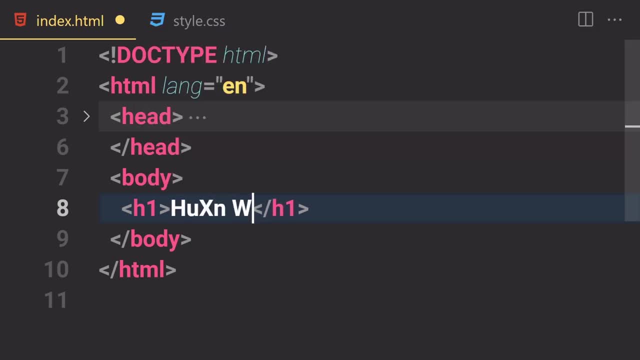 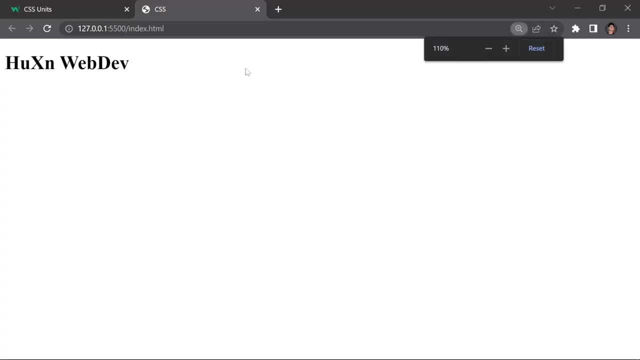 i'll do. i'll just write h1 of like husein, right here, and you should see that you can see something here right here: hosan web dev. you can write your own name if you want to. and now, if i send my file and you already what we will get inside a browser, we will get just like hosan web dev. okay, so we are. 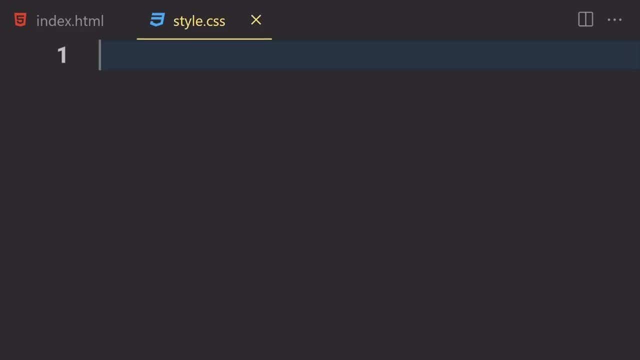 going to be starting from a typography section by first of all learning about a font family. okay, so, what is a font family? a font family will be just a look and feel of your phone. okay, so how your font will look like. so, by default, once you write your code, like by default, browser will provide a será. 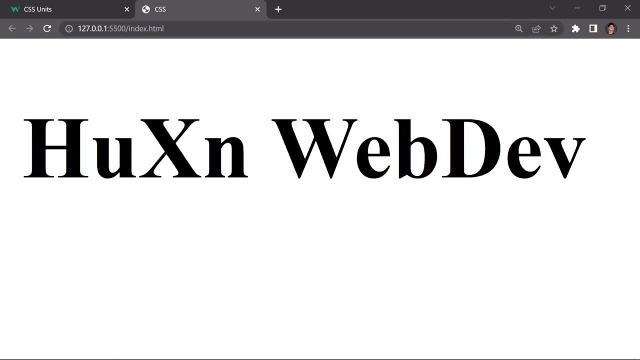 font strut. so what is a set of font? a set of font is that form which have these caps on it. so here you can see that cap, this underneath cap, and you can also see that cap on the u. you can also see it on x and n, and we don't have any caps on e right here, but we also have these caps, so these 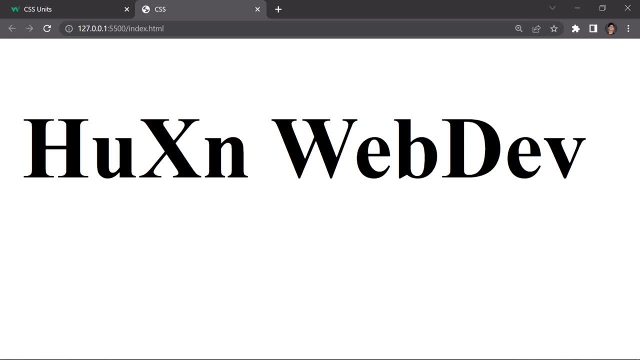 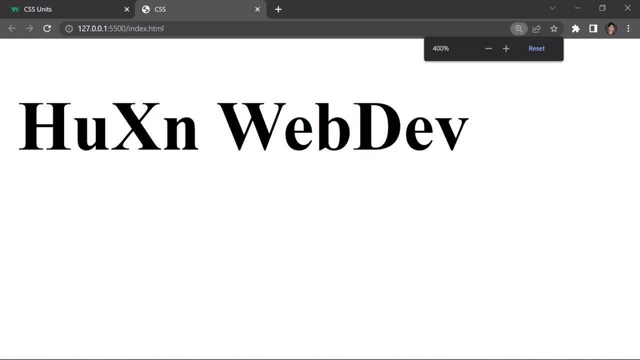 are called serifs. okay, you can call it like caps, or you can also call it like caps. okay, it a real name, which is a cap, i mean, which is a serifs, to be precise. okay, so now, by default, our font looks like this: if you want to remove this cap, so for that we can use a font. family of: 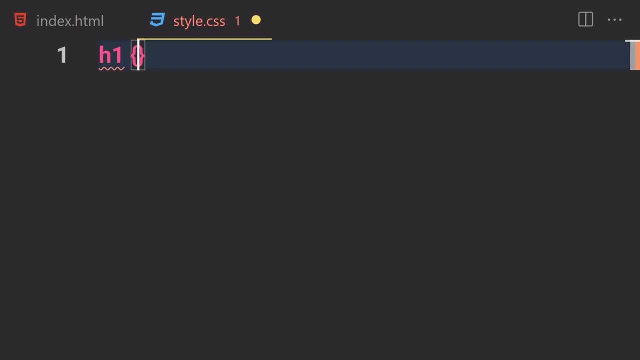 sans serif, so it will not remove that. so if you just write h1 and if you write like a font family- and we have a lot of font families in our site and we can work with that- i'm going to show everything just a second. if you just write like serif, in this case, and if you save that here you 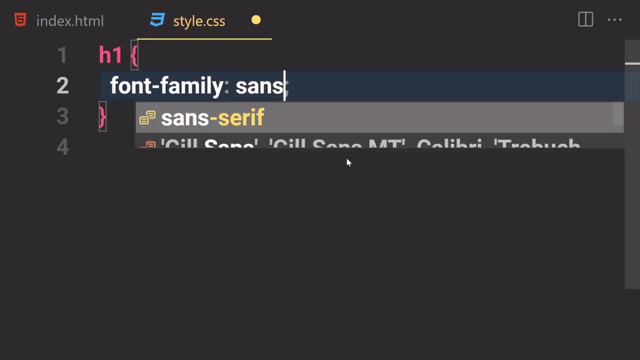 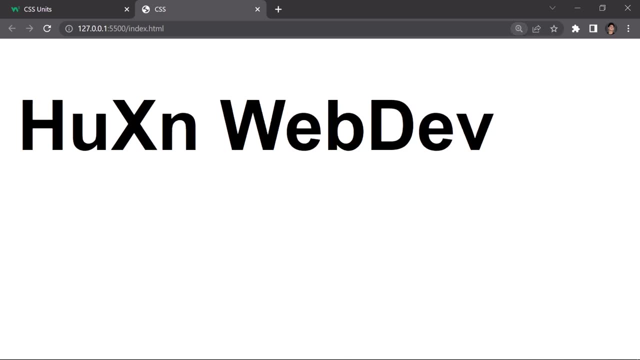 can see, nothing will happen. and if you just write like sans serif and if we save our file and here you can see that caps are gone from our font right here, and here you can see we don't have any caps whatsoever, or serif to be precise, we don't have that serifs right here, so that's gone and by. 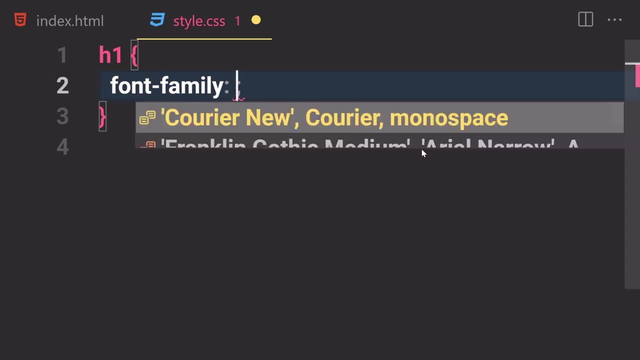 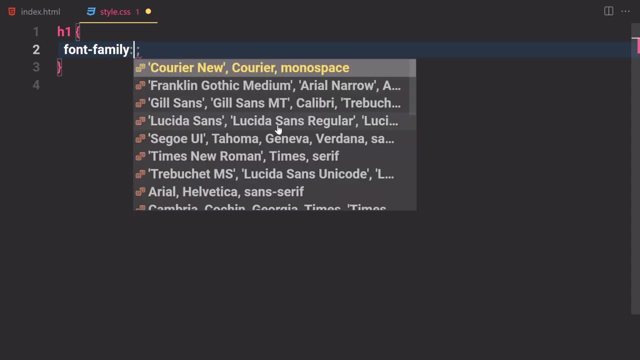 default, it will give us all of the font if you hold ctrl and hit space. so by default it will give us all of the list of the font which we currently have inside our machine if you hit ctrl space. so these are all the fonts which are currently available in my 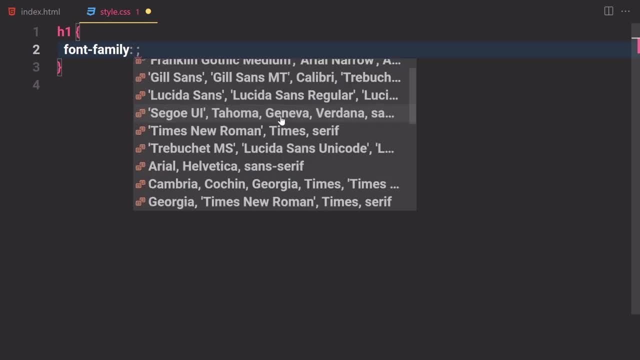 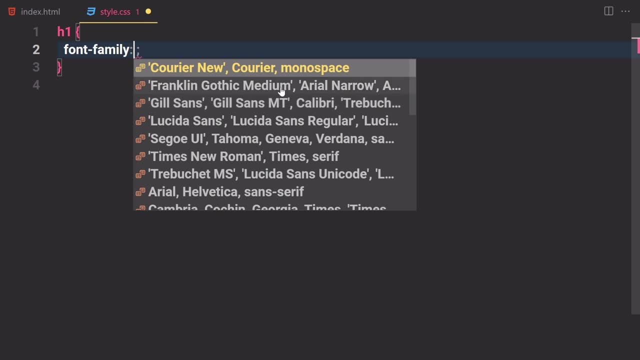 machine. so the chances are your machine will not have all of these fonts, so you can install that into your machine or you can just quickly copy that from google, which i'm going to show you just in a second. but let's suppose if i just click on this one like maybe franklin or whatever is this? 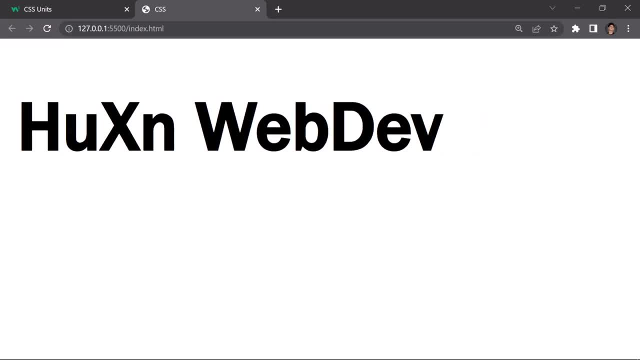 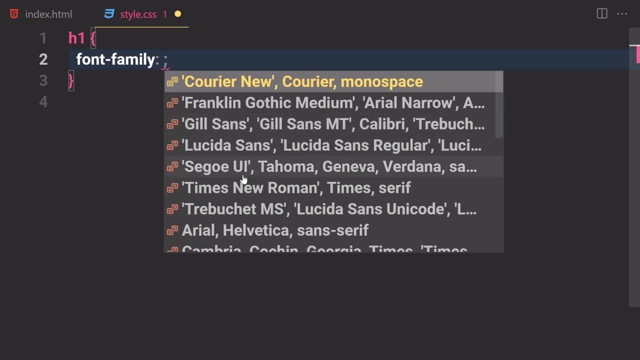 name. so i'm going to click on this one. and now, if you save my file and here you can see, this font will change to this kind of franklin or whatever the font name is. and now, if you hit ctrl space one more time, we have this seagoo ui and then we have a lot of 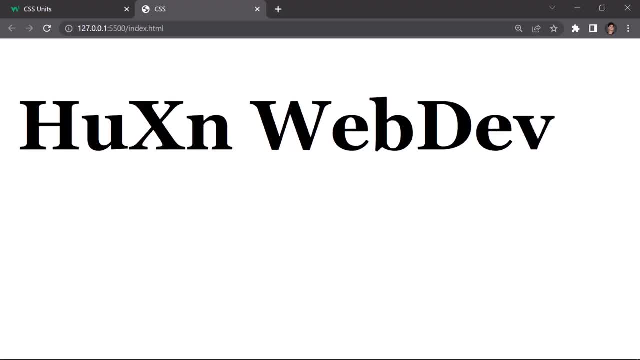 georgia. if you select georgia and save our file and georgia will look kind of like a sans serif. it is a sans serif, but it is a little bit different than that. if you just like comment this line out and if you save that- and this is how a default one looks like- and if you just uncomment that, 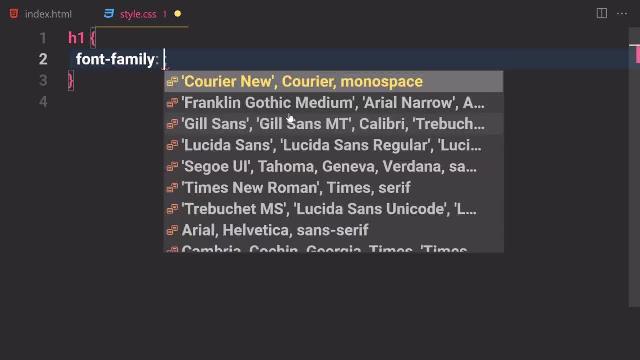 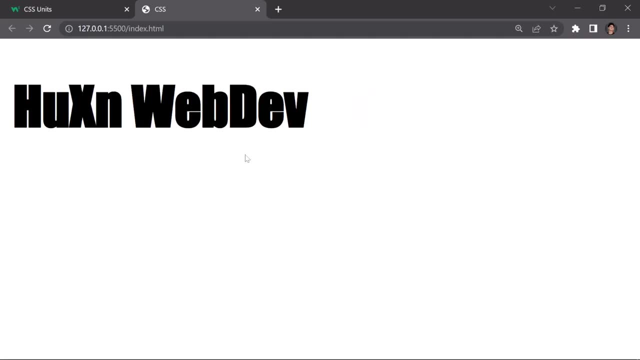 and if you save that, and this is how this georgia will look like, i'm going to remove that. we have different kind of fonts, like we have, uh, curve fantasy. so if i just click on the fantasy one and save that, and this is how the fantasy phone will look like if you select just this curve one, 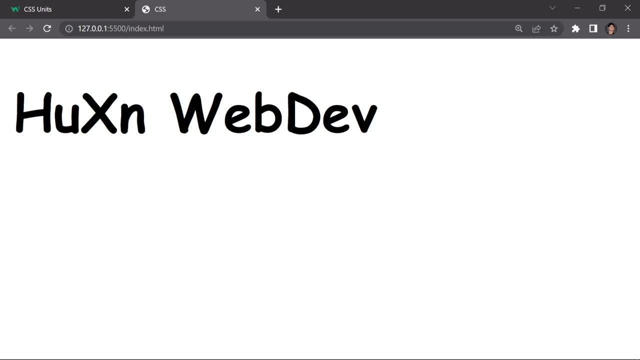 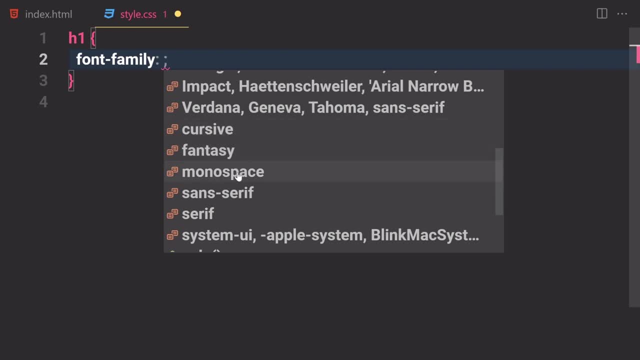 where is there and if you save that and this is how the kind of cartoonish font will look like. it's kind of like cartoonish font if you want to build application for some children, so you can use that. we have a monospace. if you click on that and save it and this is how the monospace font will. 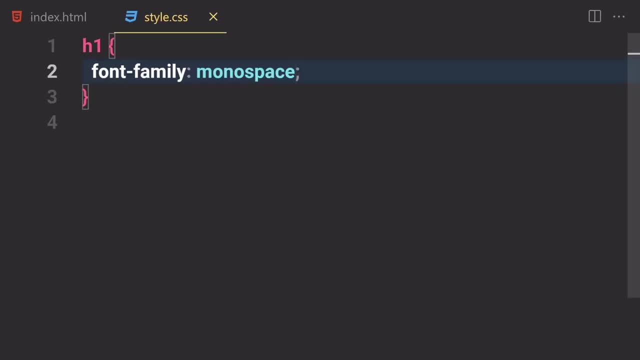 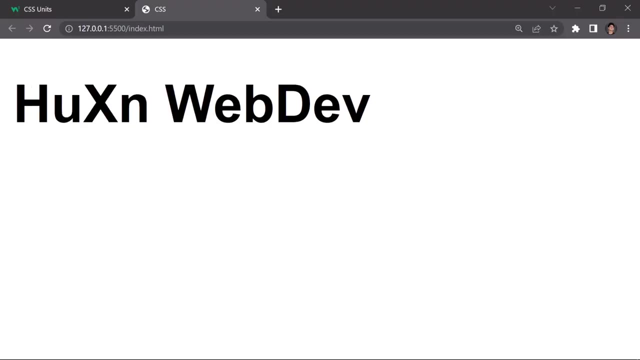 look like: okay, so this is the first thing like how our font will look and feel like. so we have font family for that, so i'm going to just change that to like sans serif seven and we just remove their serifs from our font. okay, so now the next property which i want to talk to you about in 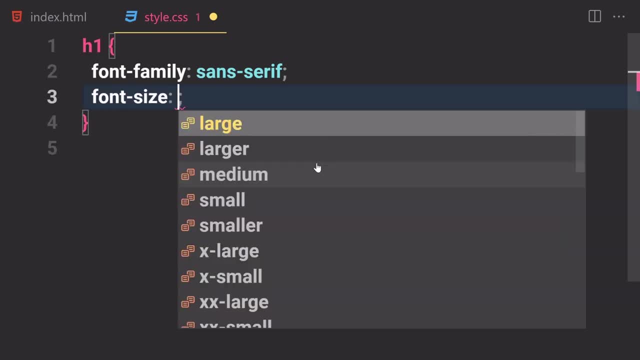 topography section is something called a font size, which we already learned. so here you can specify like: uh, by default our font will font size will be 16 pixel, and you can increase or decrease that if you want to. so like, let's suppose, if you just write like 20 pixel and if you save that and boom. 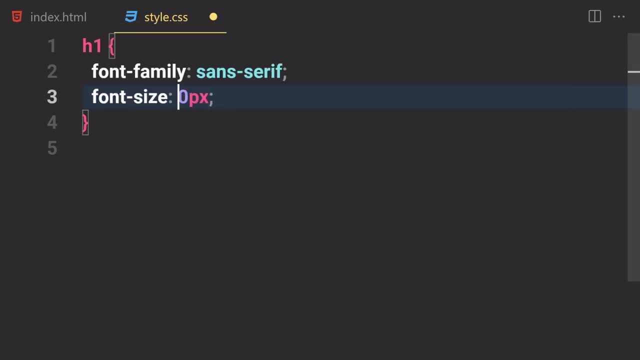 it will not use us like 20 pixel if you just want to bump it up like more, maybe 50 pixel. and if you save that and here you can see you have now this 50 pixel font right here, you can see that you have now this 50 pixel font right here. so if you save that and boom it will. 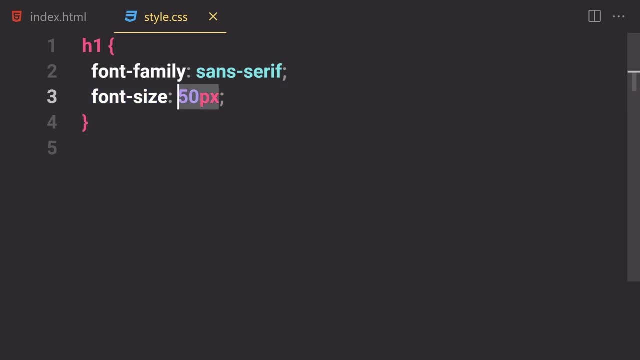 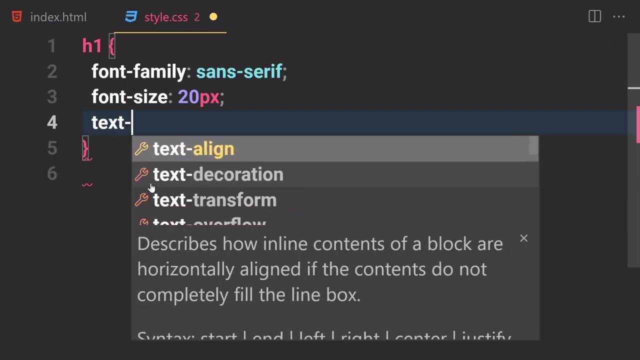 okay, and you can play around with the rems value and the ms value and so on and so forth if you want to, but i want you to just notice like we have this font size property which allows us to increase or decrease the size of our font. okay, so now the next property we have is something called a text. 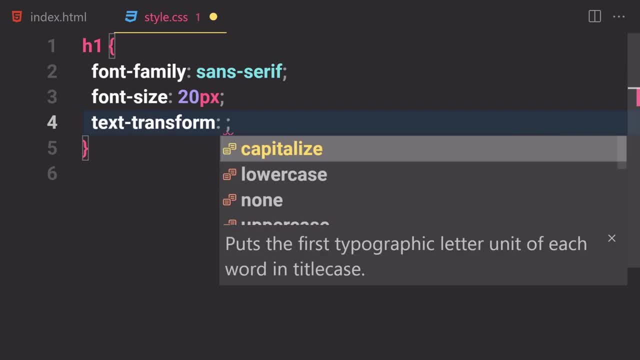 transform. so text transform will have a few values. so we have capitalized, we have lowercase, we have, uh, uppercase, which you can see here inside this list. but let's suppose, if i just click on this lowercase form and i want to change the font size, so i'm going to change the font size and i'm going 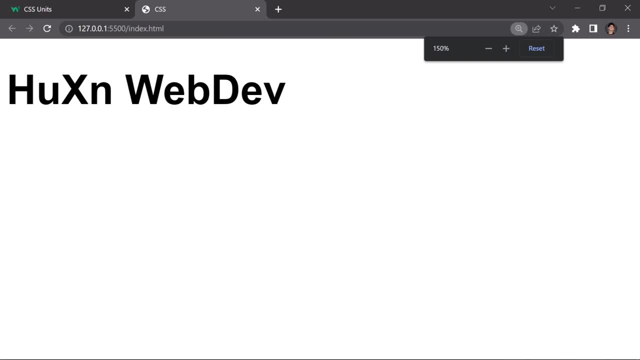 to change the font size and i'm going to use the lowercase. for some reason by default. i just wrote my phone like this, so it will just change the cases of our phone. okay, so if you save there and here, you can see all of my phone is now at the lowercase. h is lowercasses. uh, u is yellow. case x is lowercase. 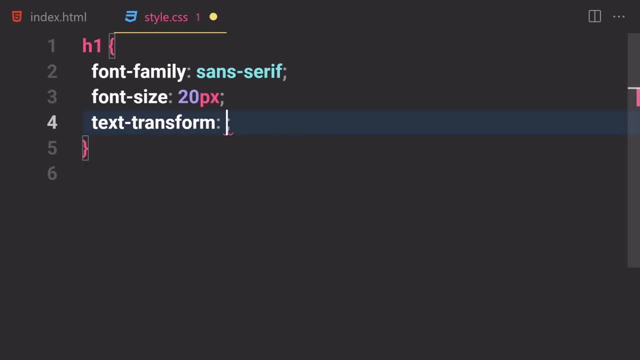 and is lowercase and so on and so forth. okay, so if i just write like uppercase, if i write like uppercase and now if you sell there and here, you can see everything is now totally at the uppercase. if you want to write like for, uh, maybe capitalize so for that we have tried more than one word. you. 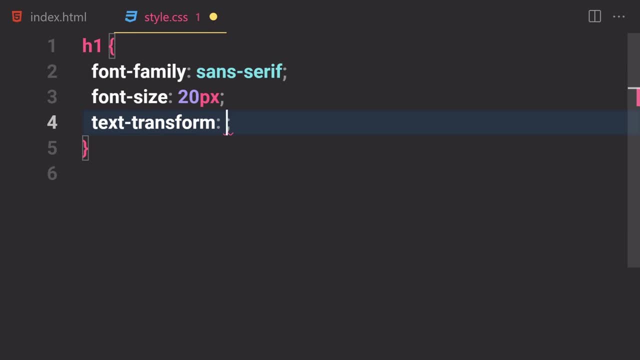 you know what I'm going to just write like text decoration or text transform off. Yeah, you know. first of all, let me just write like who's an web dev. What kind of myself is a YouTuber? I'm going to just write like a YouTuber: y o u t u b e r. So now here. 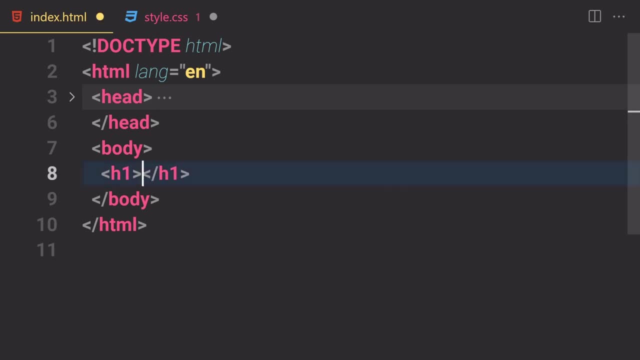 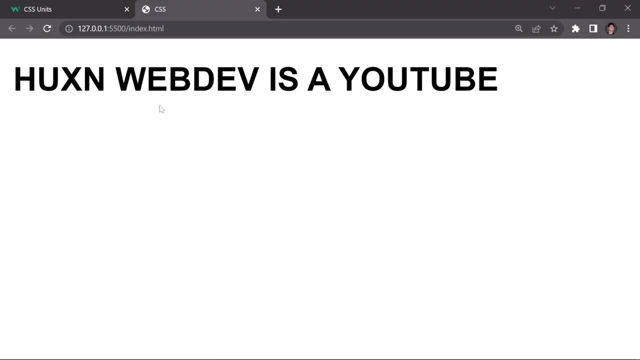 I want you to notice, or you know, I'm going to remove every, all of them, And here I'm going to just try, like: who's an is a hosan web dev is a YouTuber, Okay, so if you sell that. so here you can see, everything is now perfectly at the uppercase, And here we wrote. 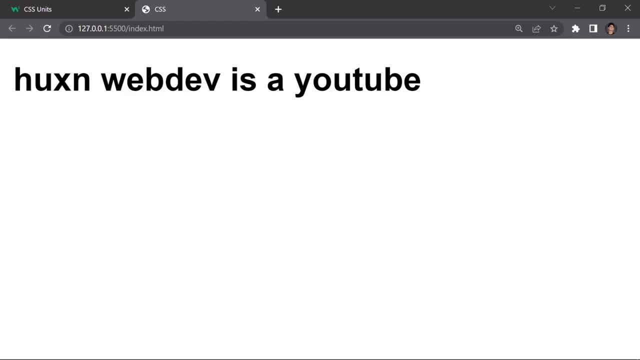 that as lowercase. But if you just save this file here you can see everything is now at the lowercase right here. But if you want to change that to capitalize, so capitalize will just uppercase the first letter of the word, like this: H will be uppercase this W. 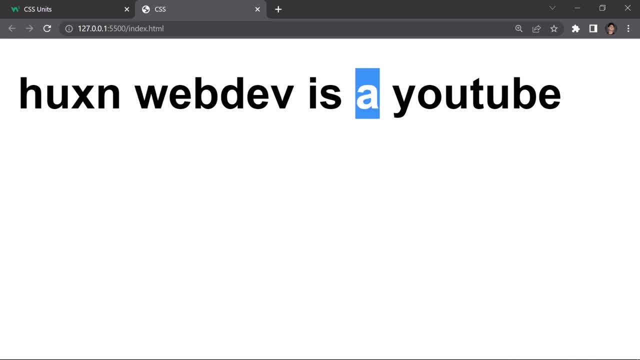 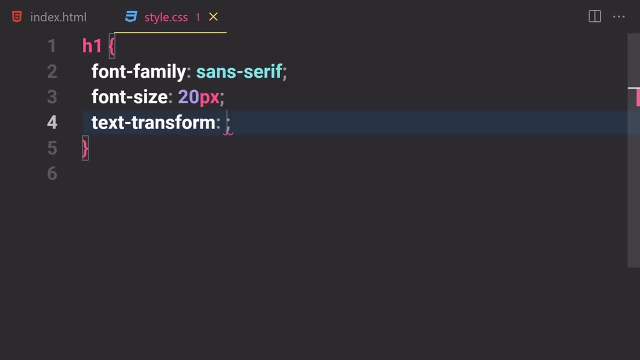 will be uppercase, I will be uppercase, I guess I will be uppercase, and Y will be also uppercase And the rest of them will be lowercase. Okay, so this is what capitalize will do for us. So if you just try like capitalizing here, if you sell that and now here you can see. 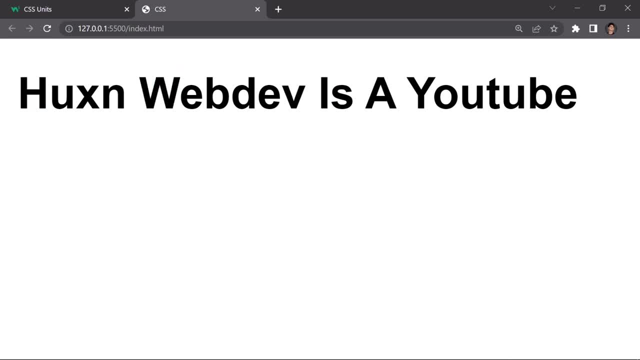 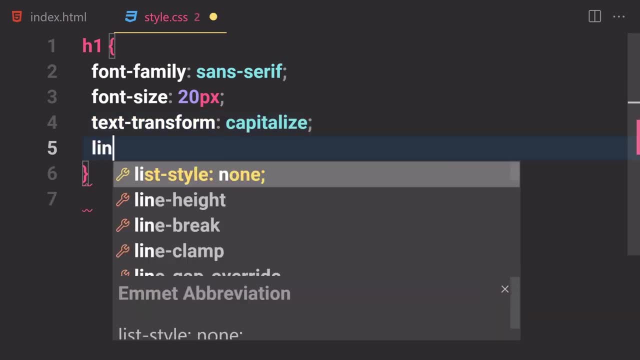 every letter of the word will be uppercase and the rest of them will be lowercase. Okay, so this is a text transform property. And now the next property which I'm going to explain is a line height. So if you want to explain a line height, you know. first of all let 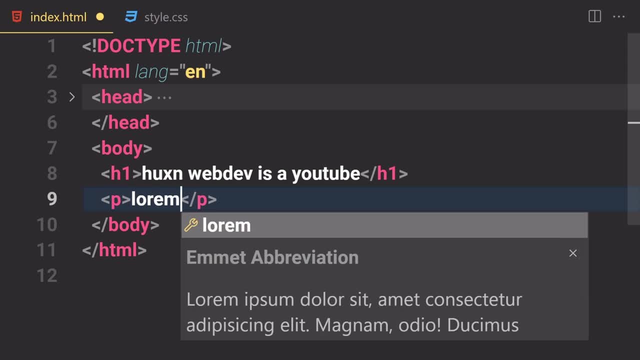 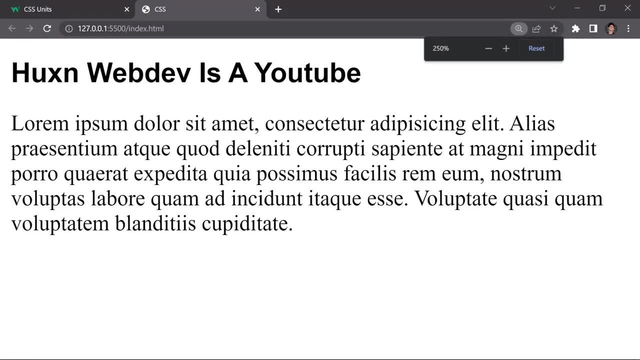 me just write a paragraph in here: lorem of maybe- I don't know- 40 will be fine. I'm going to write lorem 40. And if you sell a file and now here you can see, by default we get like this: 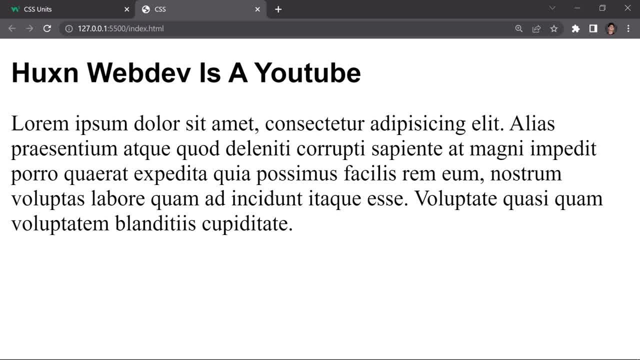 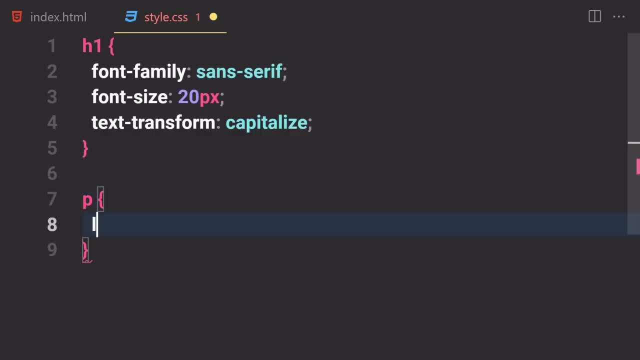 little bit line height right here. But if you want to increase these line heights, so for that we can write, or on CSS. So I'm going to now select this paragraph right here And here I'm going to just provide like line height, And what is the line height we have to specify. 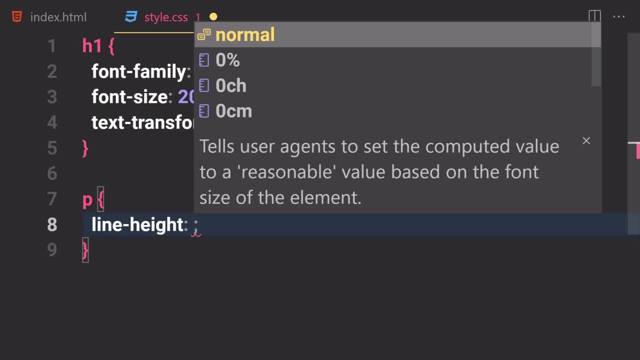 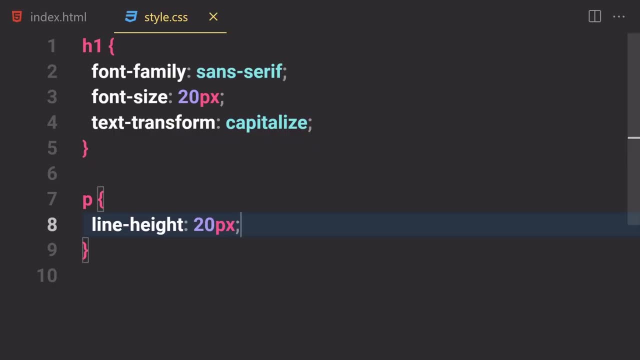 some property, like some value, inside this line height Maybe if I want to write like 20 pixels, if I just write 20 pixels, if we sell that, and here you can see, it will just decrease that a little bit. And if you want to increase that like 40, and if you sell that, and here you can see, 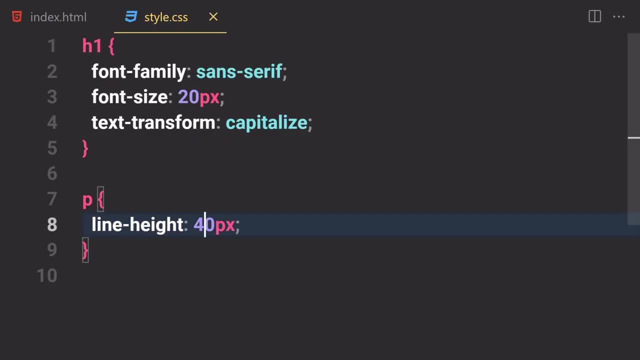 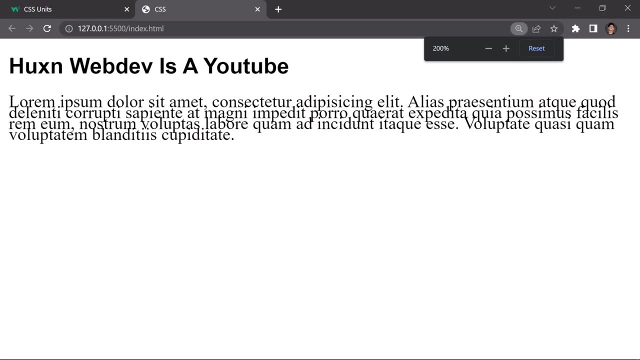 it will just provide a line height. inside this line, If you want to write like 60,, seven and this, how it will look like. if you want to try, like maybe 10.. So if you sell that and we'll just jam it in together. And if you want to go lower than that, so you can. 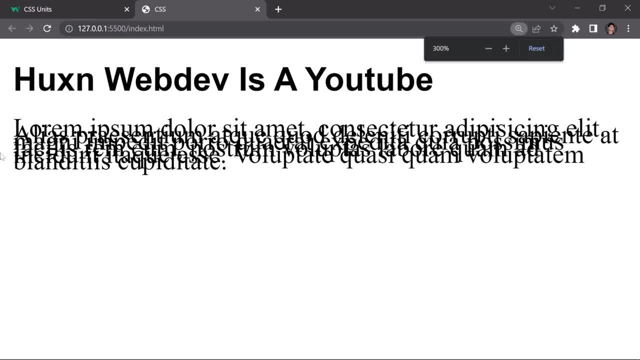 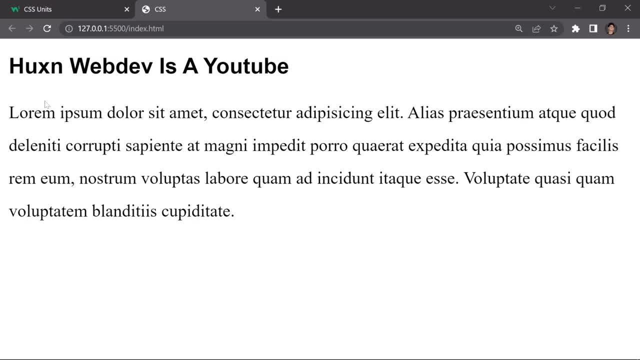 just write like four and fissao there And for just look horrible, right? Okay, so you can play around with that if you want to. I'm going to just stick to like 30.. And now if you sell that- and this is how it looks like right here, And now if you want to increase. 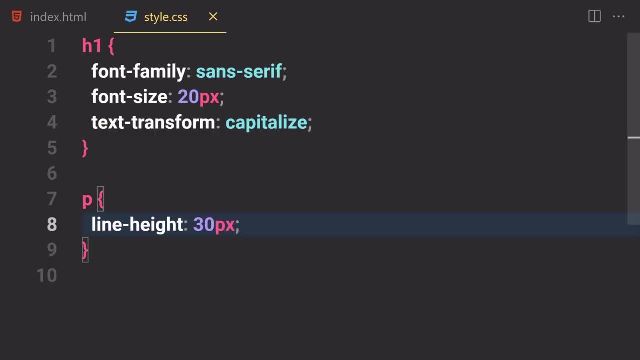 it like 40, and if you sell that and if you want to just jam it in together And if you right here, okay, so this is a line hide property. a line hide property will just allows us to provide a hide inside a line, either increase that or decrease that. then we have a letter spacing. so 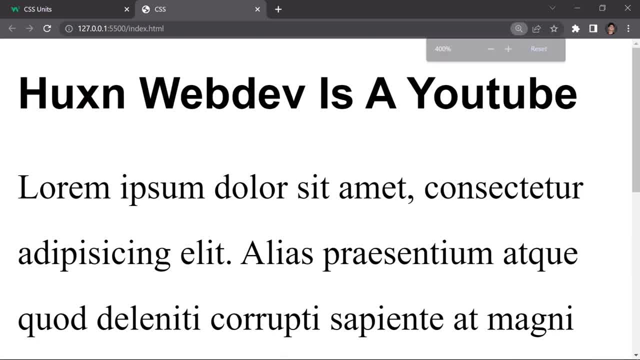 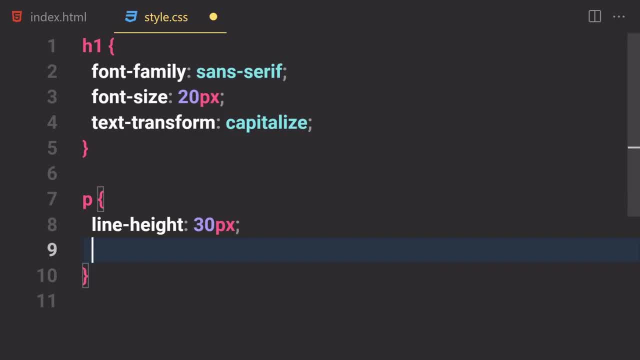 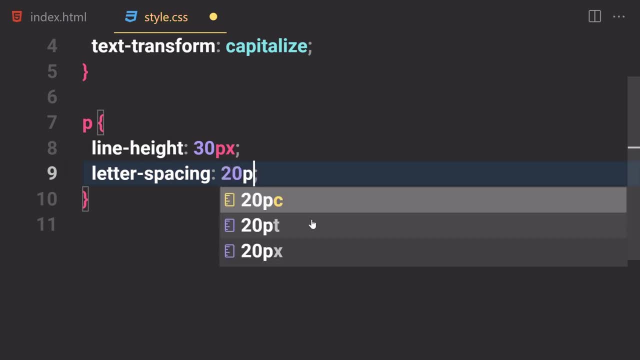 if you want to get a spacing inside this letter, so if you want to get a space inside this l o o r e m, so if you want to get a space inside there, so for that we can just write like um letter spacing. and here we have to specify how much spacing do we want. so we can just write like 20 pixel space. 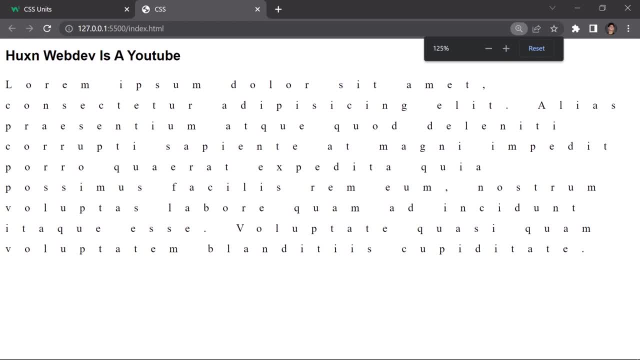 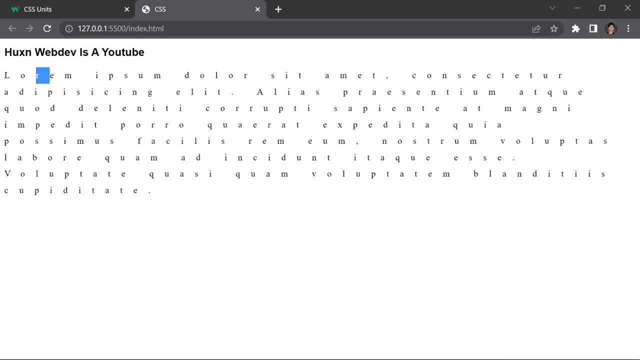 it will be a little bit huge. so if you save that- and this is how it looks like right here- okay, kind of awful, but here you can see we have 20 pixel space in here, 20 pixel in here, 20 pixel there and so on and so forth, we can also decrease that by just writing like: maybe five and okay, so it's. 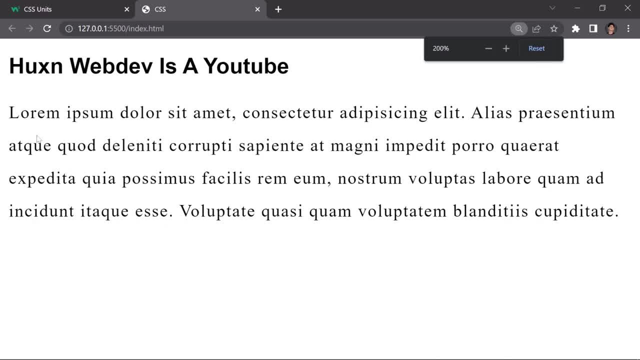 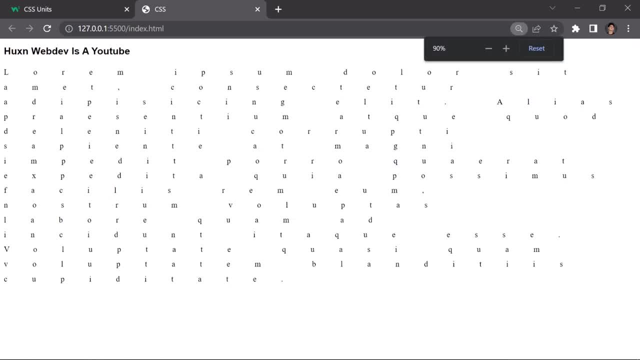 also a little bit. you just write one and one is the default one. all right, so we can just write like maybe 50 if you want to and if you save that, and this is looking horrible, this is looking totally horrible. so we can just do crazy stuff like that by using css. i'm going to just remove that, you know, i'm going to comment. 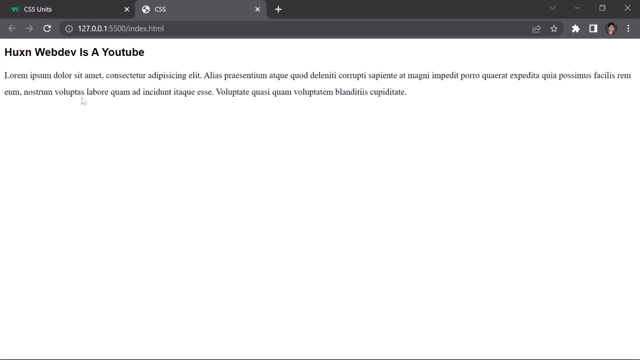 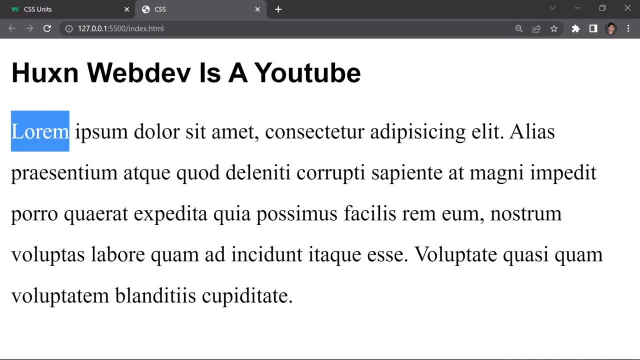 it off so you guys can see everything a bit better, all right. so now, if you want to get a spacing between each letter, so not not a letter, but in a word- so now, if you want to get a spacing between this l o o r e m and this ipsum, like in this area, so for that we are going to be writing a word. 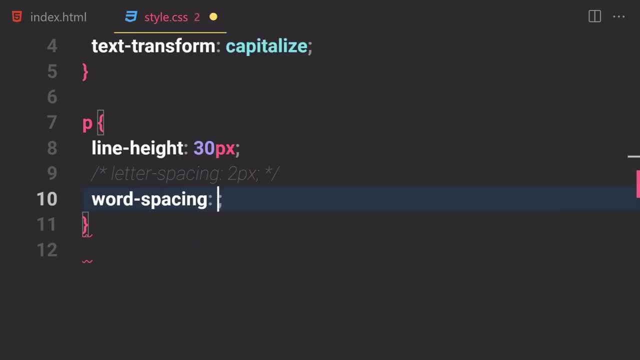 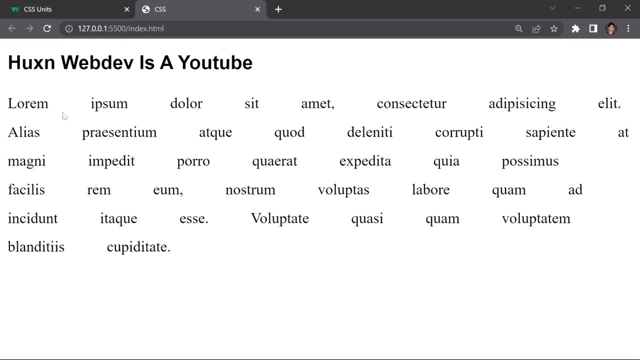 spacing. so i'm going to just write like word spacing, okay, and here we have to specify some value to it. so in my case i'm going to just write like 40 pixels. if we save that, it will not provide spacing between our words right here, okay. so if i just 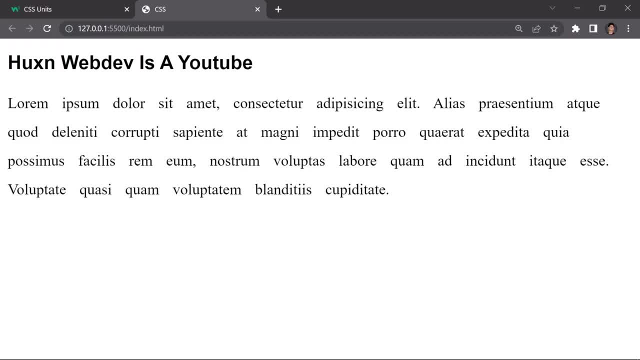 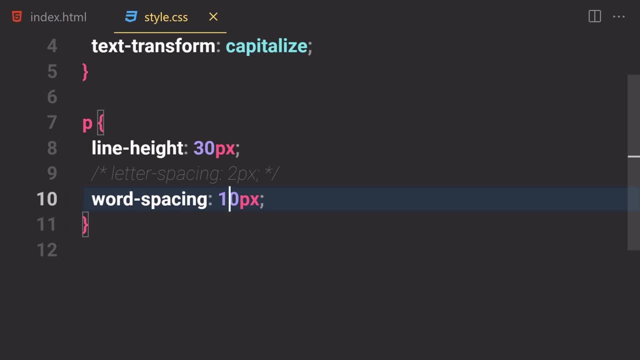 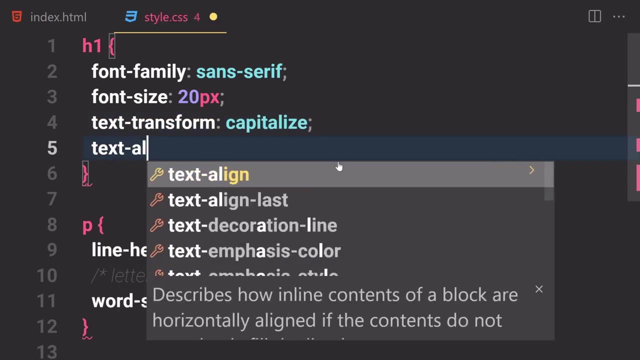 want to write like 20. i'm not provided 20. 10 and 10 will look like this and you can play around with that if you want to. okay, so now let me just write a text align property, so a text align will just as the name suggests, it will align, or text. so if you just write like text align property and 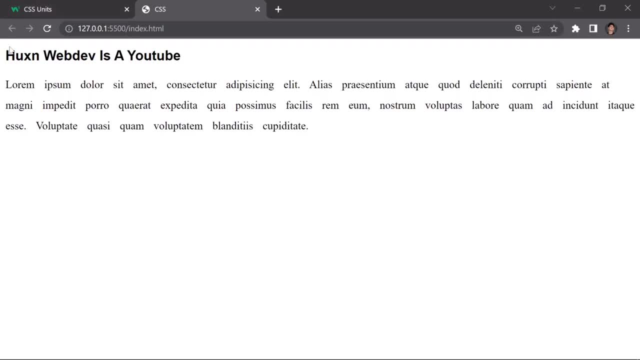 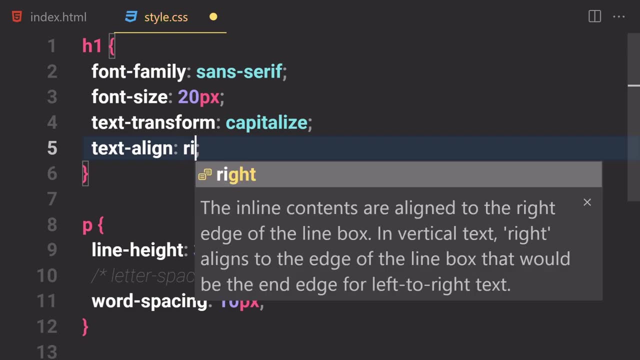 by default it will be set to left. so if you just save that and here you can see, by default it will be set to right here. if you want to push this to a right, so we can just write like our text line of right. and if we save that and here you can see, our text is now went from left to right- right here. 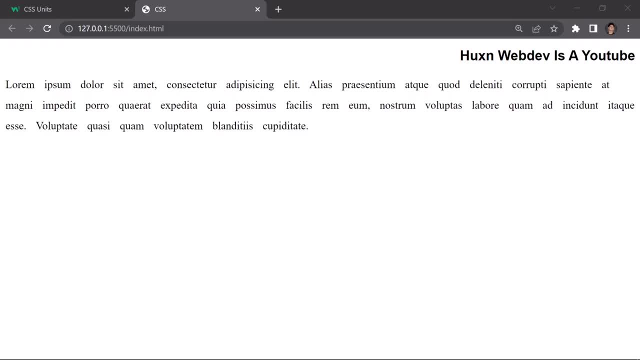 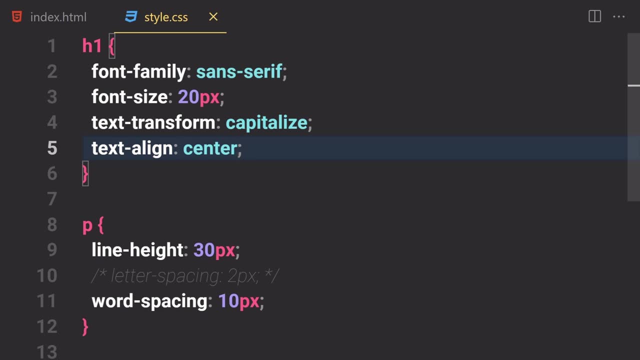 if you want to make that center, so for that we can just write like center. and if you save that and here you can see, our text is now it perfectly at the center right here. okay, so we can play around with that if you want to. and now let me just show you the text. decoration property in. 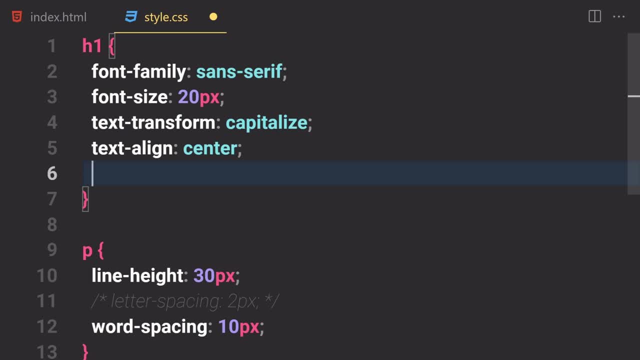 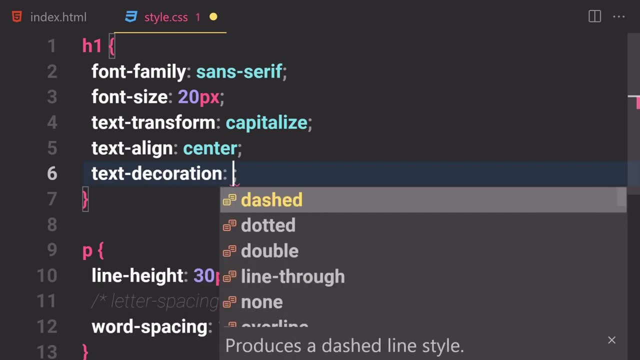 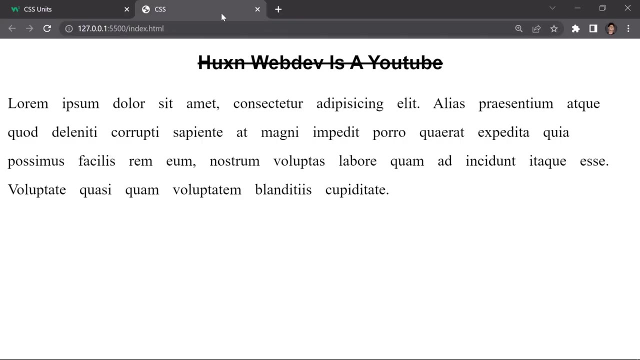 some cases you would want like decoration for underline or line through or not. you can just write a text decoration property. and here let's suppose, if you want to write like text decoration of uh, i don't know, um line through maybe. so if you save a file, so here you can see, it will not provide. 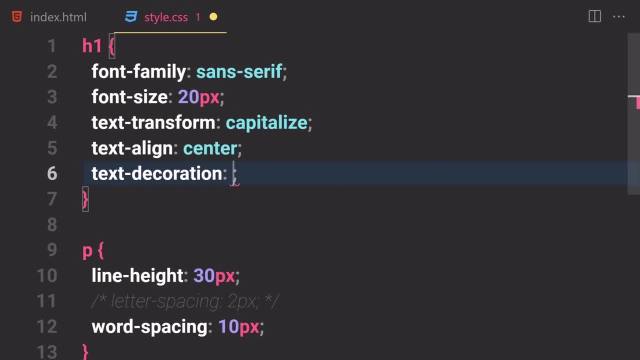 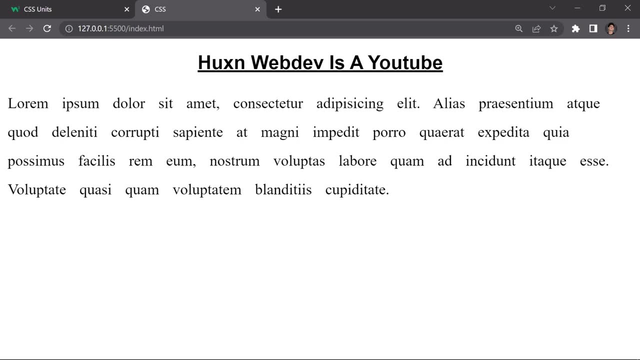 this line or text decoration like line through if you want to write like text decoration of underline, and if you save that here, you can see it will not provide this decoration as an underline right here. okay, we can also provide it to like: uh, what was the other one? let me hit ctrl space, so don't know use. 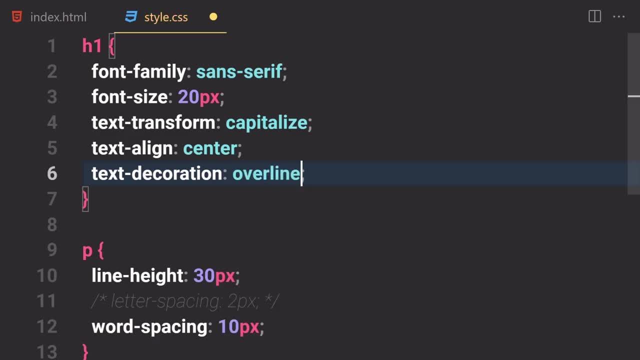 all of this value. so we have underline overlines. if we just save that, so we'll not provide the line at the top right here. okay, so this is how we can work with that. but if you want to remove that, you can also provide this text decoration of none. and if you save that, so you don't know, just remove. 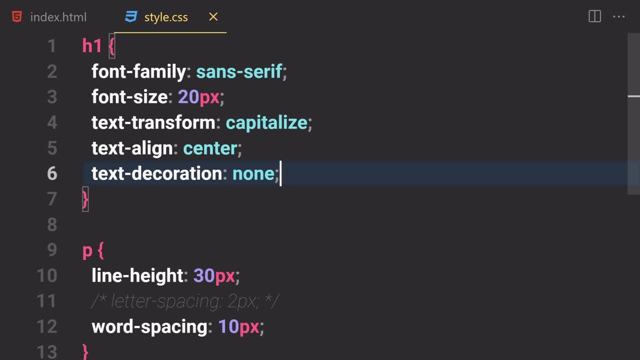 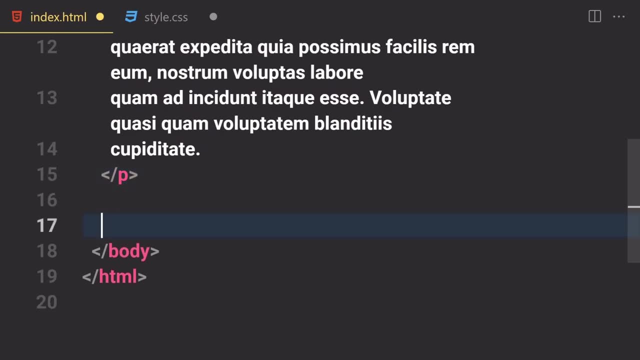 that decoration from it and this text decoration and none can be useful for anchor tags in some cases. so if i just comment off this line and if i just write like anchor tag right here, so let me just write an anchor tag and it'll go to nowhere. but if you have like i don't know, learn more and 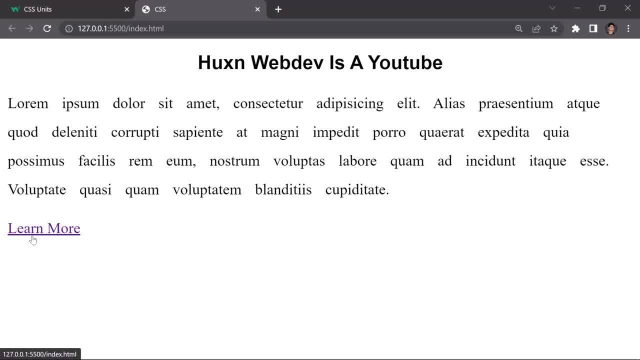 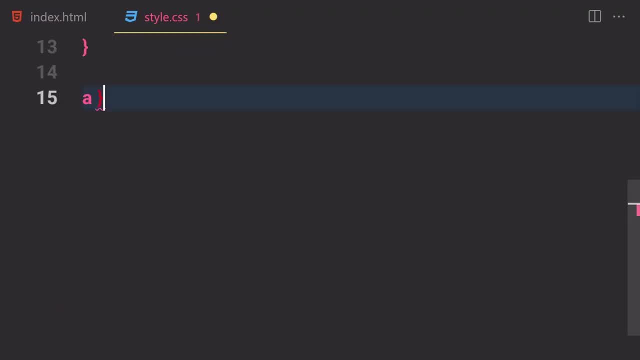 if you save that here, you can see we have text decoration of underline right here. but if you want to remove that, so for that we can just write like: first of all, let me just select my anchor tag right here, and here we are going to be just writing like text decoration of none. so if 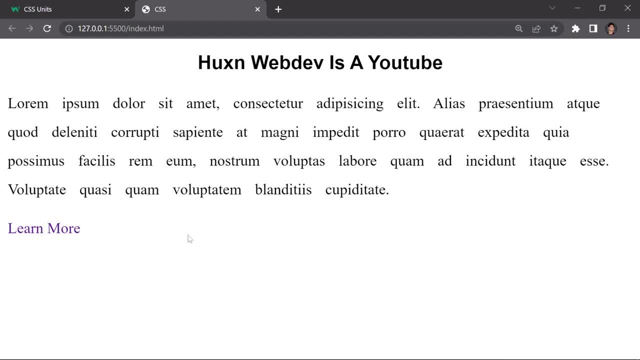 you save that and, boom, that's gone from it. okay, you can change the color if you want to. you can just write color and black and if you save that, so it will look like these, but if you hover a mouse over to it, so you would get this kind of a cursor right. 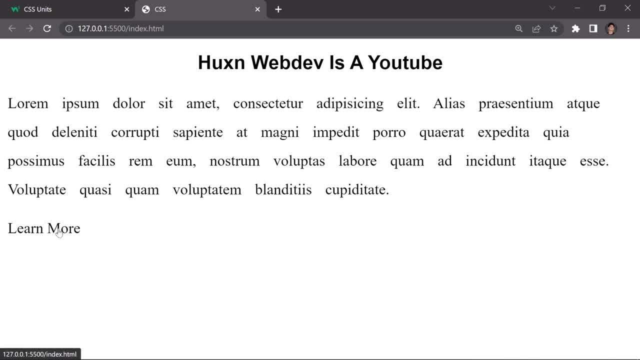 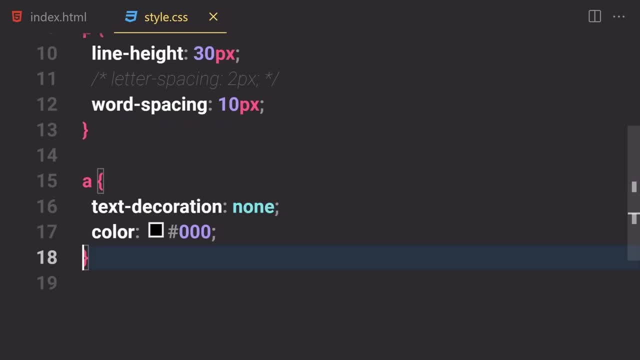 here. and, by the way, if you want to change these cursors- so you have a lot of cursors in css- so if you want to change the cursor, by default in uh anchor tag, we have, like you know what. i'm going to show you that inside a paragraph once you hover mouse over to a paragraph. so you want to. 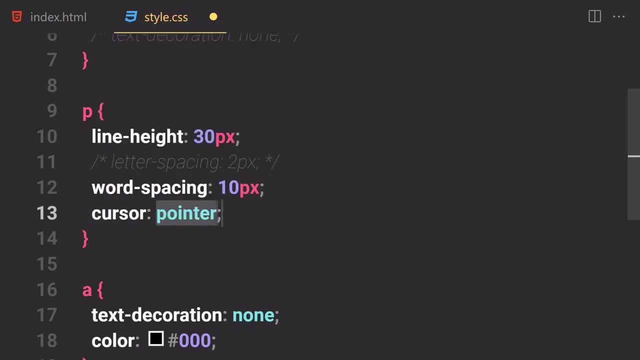 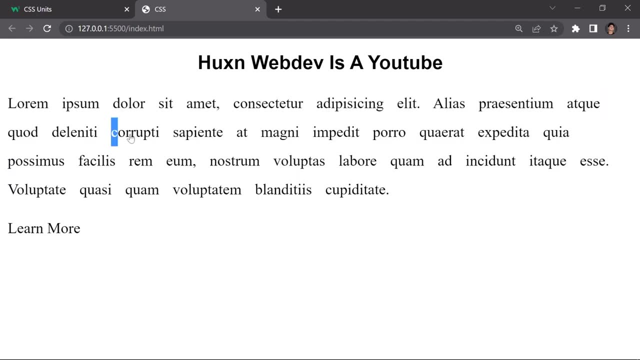 change your cursor to something else. so let's just write like cursor of pointer. so if you save that, and now if you hover mouse over through this cursor, so it will be like clickable, but we can also select everything and stuff, but it will change this cursor to this pointer right here. okay, 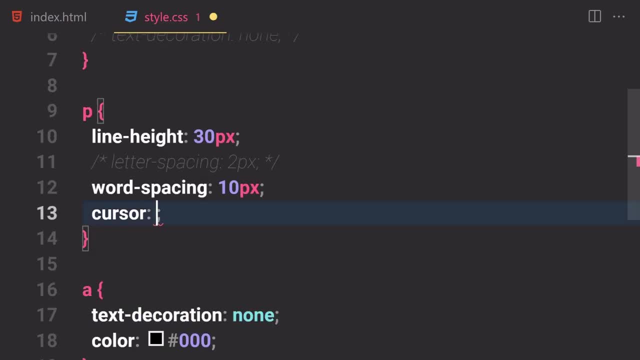 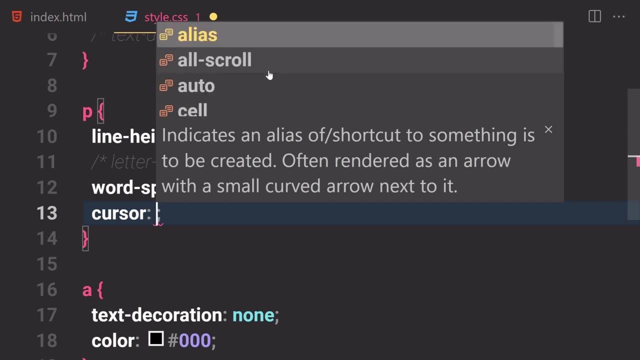 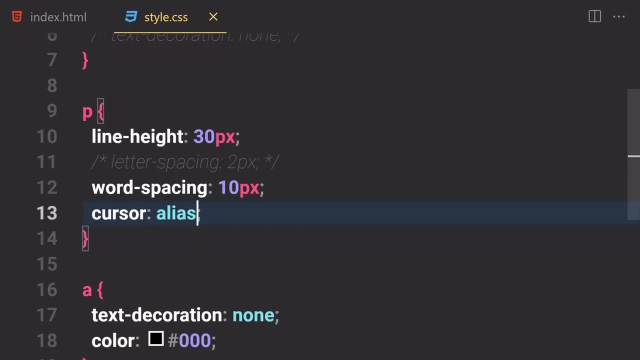 so if you just remove this pointer from there and if you hit ctrl space and we have this alt, scroll, auto and then cell and call resize, let me show you all of them just like one by one. so if you just write alias here, you can see it will not just gives us that alias kind of cursor, if you 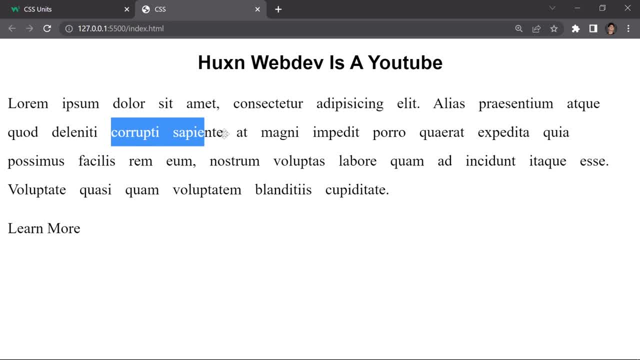 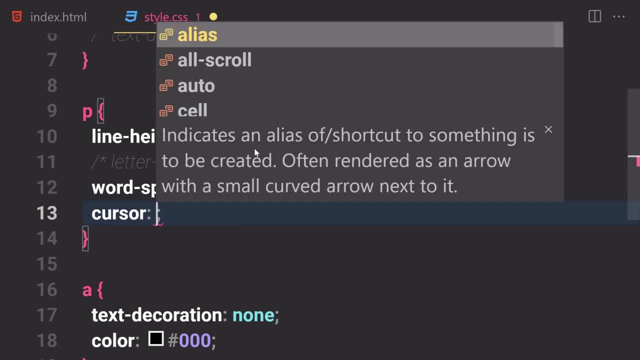 select this alt scroll and if you save that and here you can see it will not gives us this alt scroll, kind of uh circle right here. i guess you can see that, but now you would see that then we have another one, which is that auto save it and auto will be this automatic one, and then we have 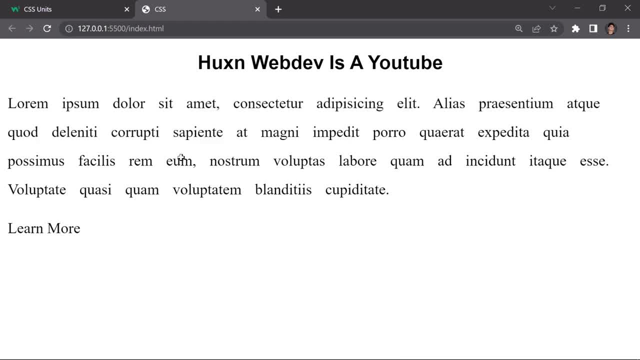 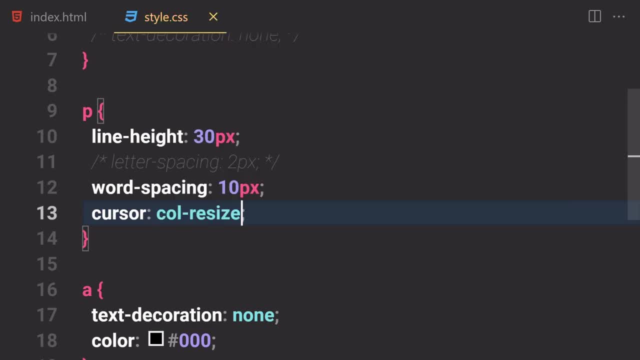 this cell if you save that, and this is how it will look like kind of a plus sign if you never used that before. and then we have a different kind of like called resize, if you save that, so it allows us to like resize our stuff. and here you can also see this cursor right here we have 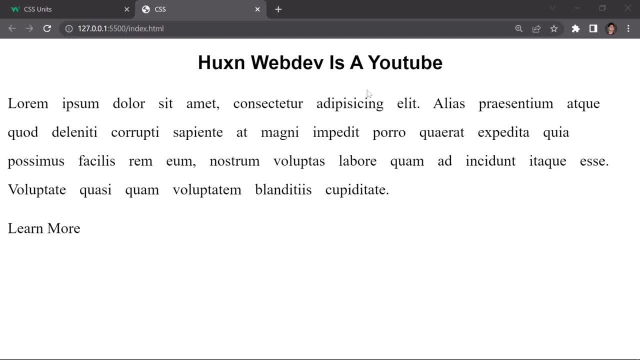 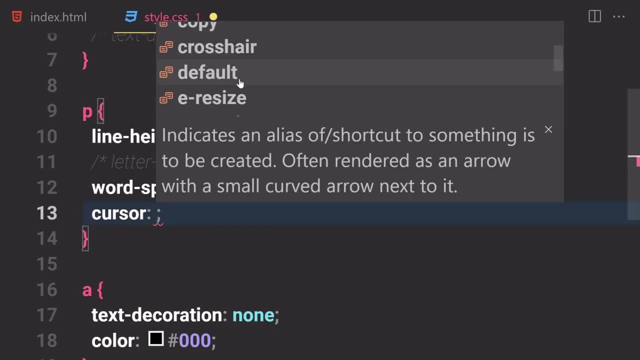 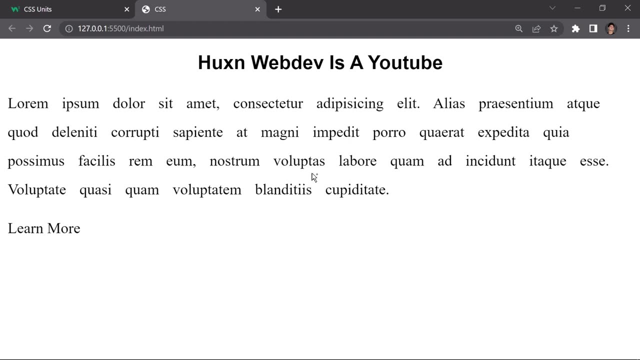 definitely different kinds of cursors, like uh context menu, and i guess i've never worked with this context menu one, so i'm going to remove that and now let's just select or copy one. so if you save that and now here you can see, it allows us to like, copy some text, and here you can see that plus symbol. 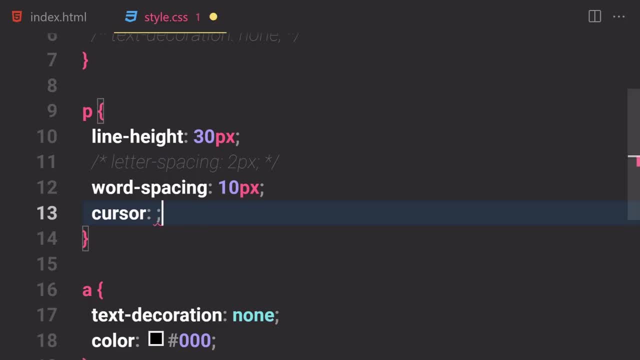 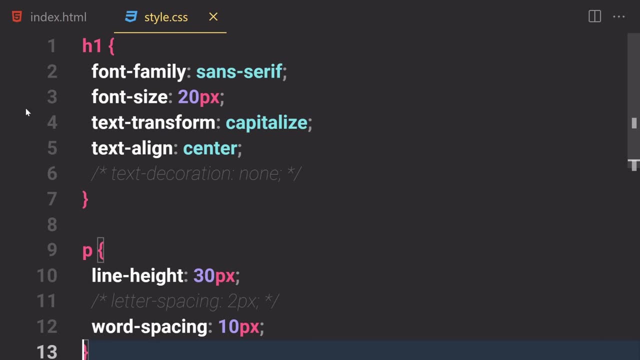 okay, so you can see that you can play around with the cursor if you want to, but i'm going to just stop from a cursor right now. all right, so now that we know enough about typography in css, like we have font family, font size, text transform, text line, text decoration, line height, letter spacing. 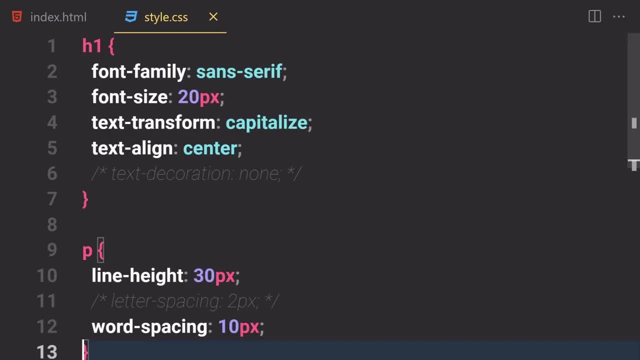 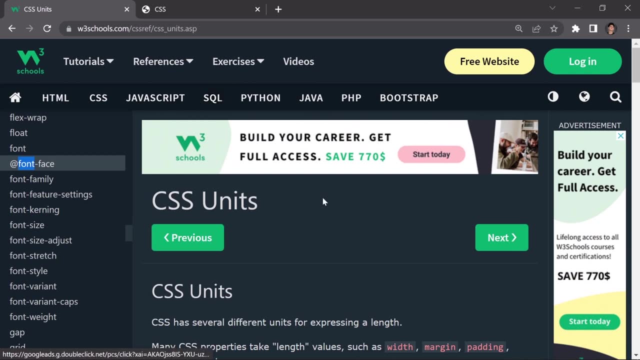 word spacing and so on and so forth. now the next thing which i want to show you: in some side you would say, like great fonts, like uh, there is a great font using this site. but in some side, if you visit that site and you want to get that font, so you can just right click on it and click on. 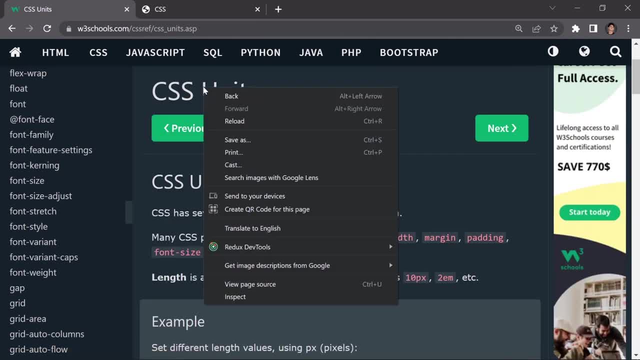 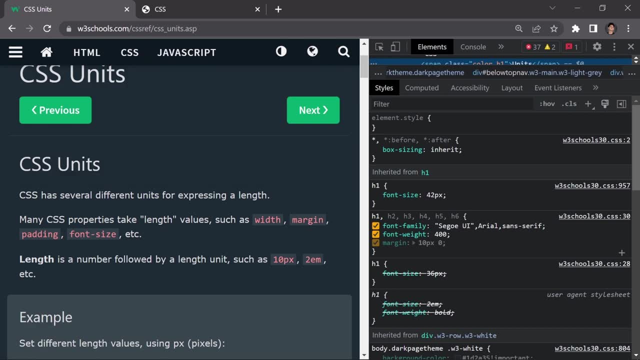 this inspect area. just right click on it somewhere and then click on this inspect area, so it'll now inspect you and it will also give you that font family. and here you can see that font failure of this seagull ui aerial, sans serif or whatever it is. 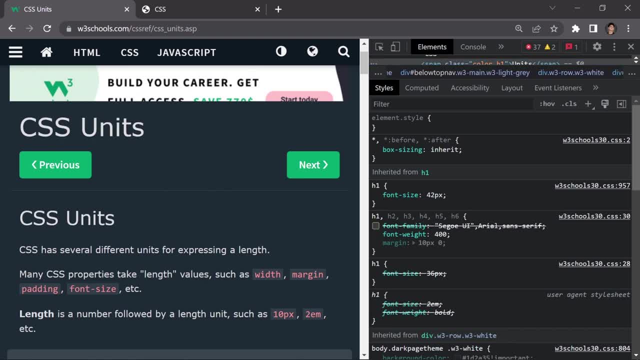 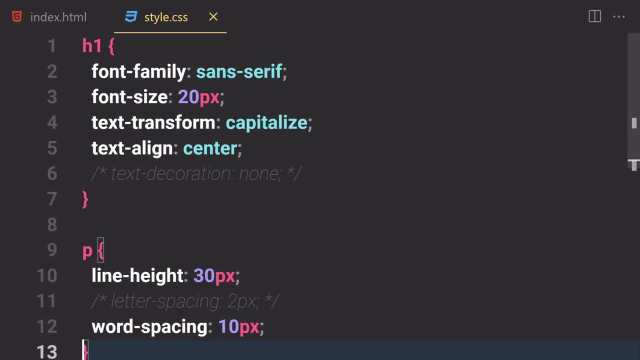 if you just uncomment that or if we uncheck that. so here you can see by default, if we use that kind of an ugly font and we have font weight and i already forgot to show you a font weight as well, so now let me just show you a font weight real quickly. so here you can see we have a font size. 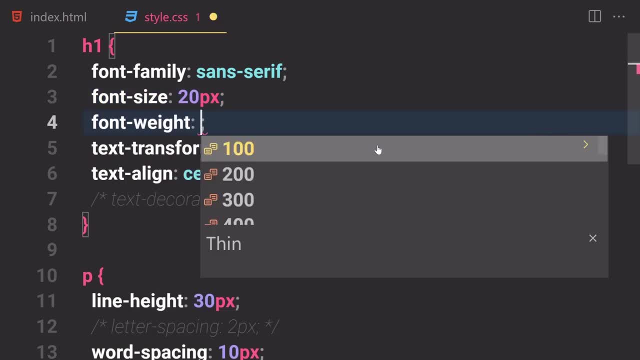 so now let me just write a font and then weight, and font weight allows us to change the weight or the boldness of our font. so by default the paragraph will have, i guess, a normal or 100 one, and if you set that to like 700, 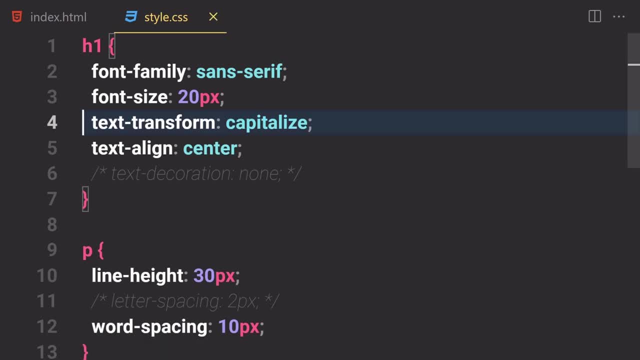 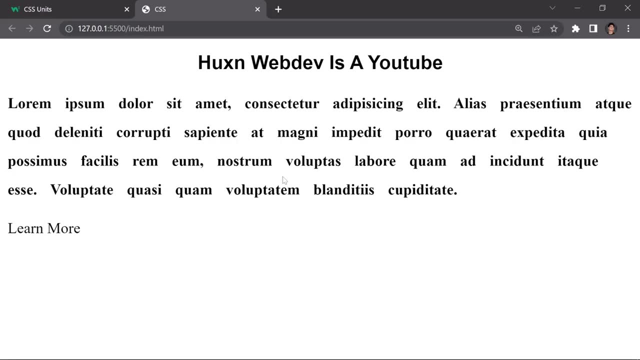 and if you save that, okay, it's not working, let me just remove that. okay, we are using that on h1. so if you just write it right here inside a font size and if you save that and here you can see, it will now set to bold right here. you can also provide, uh, different kind of values, like normal. 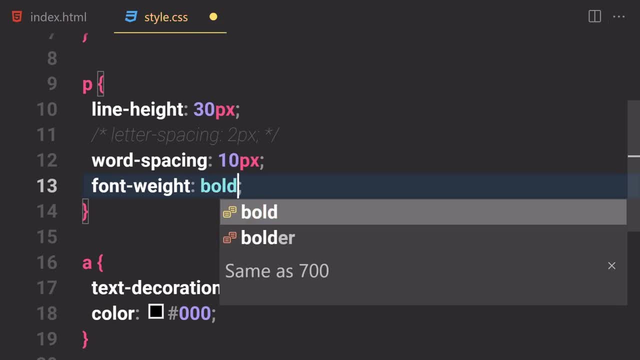 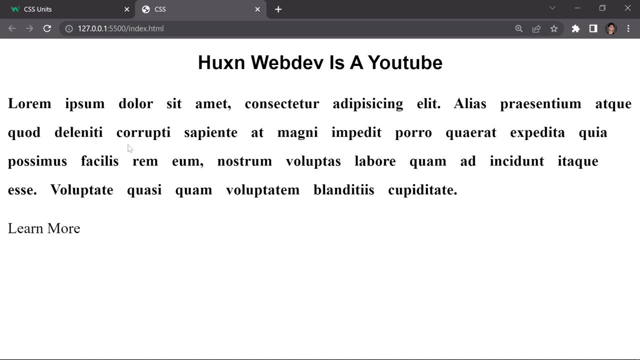 and normal will be the default one, and we can also write like bold. we save that, it will now bold if you just write like a bolder, and if you save that, it will now be like a bolder, and if you save that, so it will just be a little bit much bolder than just a simple bold one. okay, so here. 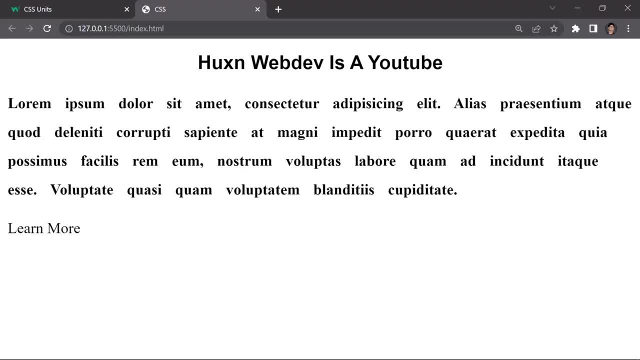 you can see inside this h1. so there h1 will be by default bold. okay. so if you want to change that to normal, so we can just write like font weight to be normal. so if you save that and here you can see, it is now become to normal right here. okay, so that was it about our typography. now the next thing: i 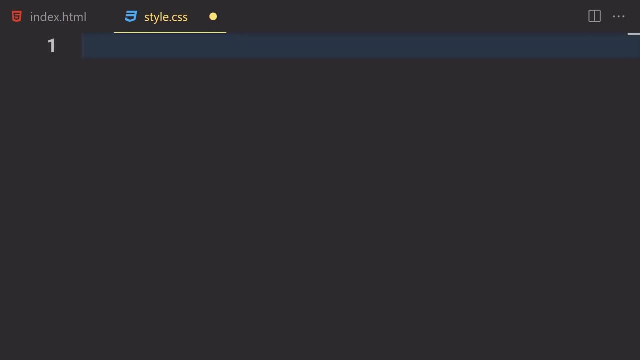 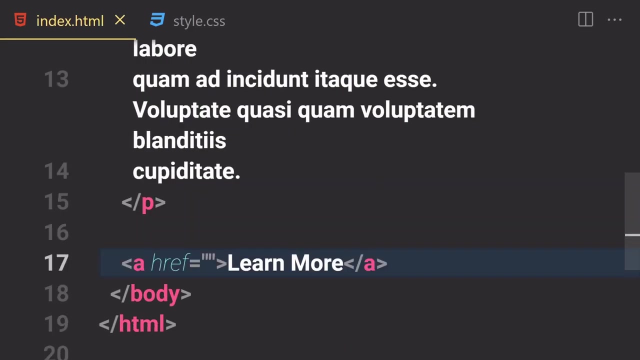 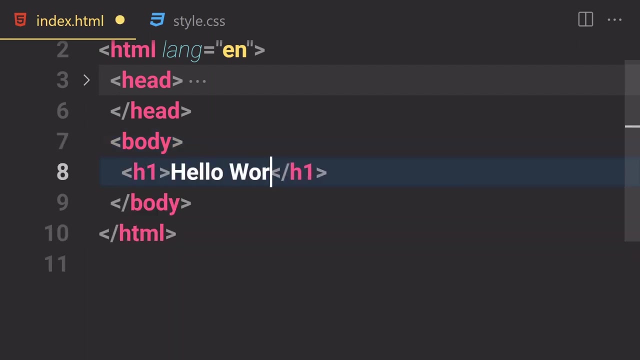 want to show you is that how you download a fonts from a google font and then you can use that inside your project, if you want to. now i'm going to remove everything and i'll send my file, and i'm also going to remove everything from a body tag as well, and here i'll just write h1 of hello world, or you know what huzzain will. 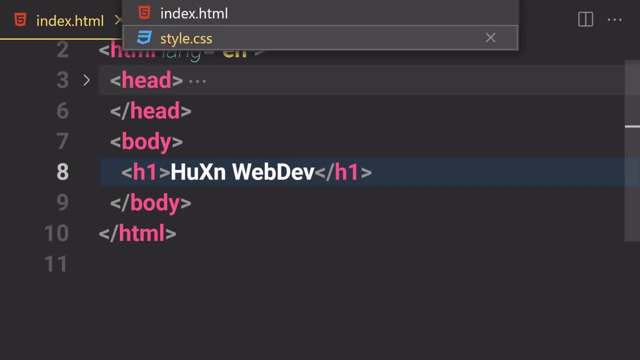 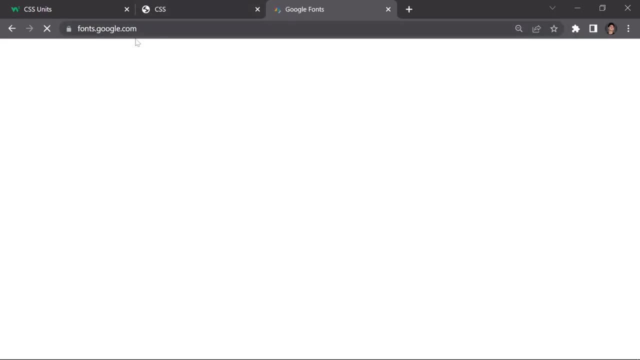 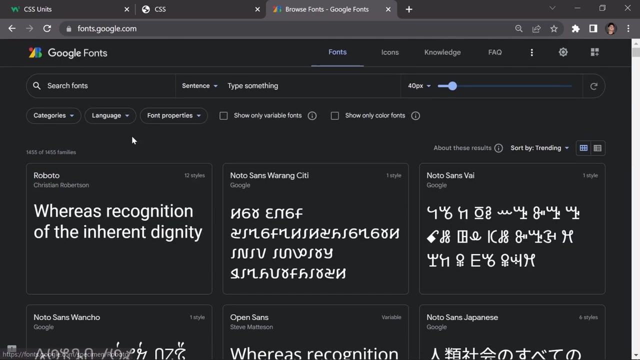 be fine, you can write your own name if you want to. so i'm going to send my file, and now what i'll do is that i'll just go to my fontsgooglecom. so you just have to write like fontsgooglecom and here you would find insane amount of fonts right here. okay, so we have like a sensor, if you. 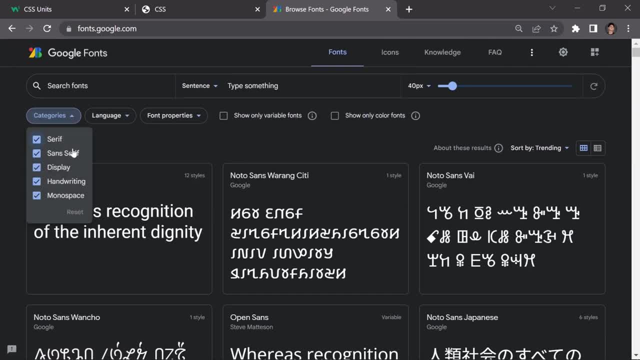 can choose the categories if you want to. if you want to get like serif form or sensor form, display form, handwritten form or monospace form, you can also change the languages. if you want to get a form for that, you can also change the form properties like uh, numbers of form and then 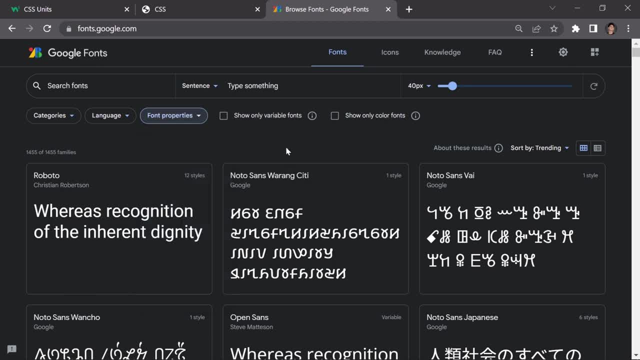 the thickness of the form, the slate, the width and so on and so forth. and this one is a new one- show only variable forms, so those forms which have a variable, and you don't have to worry about any form variables and stuff, and then show only color. 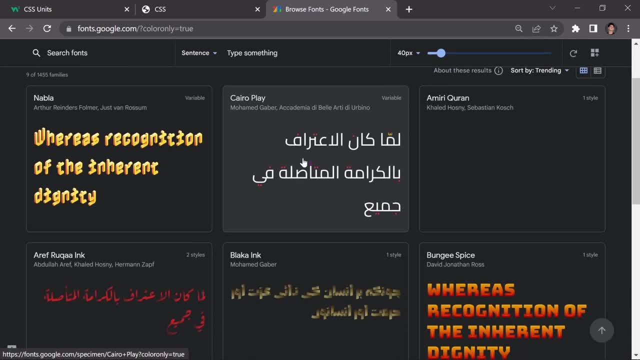 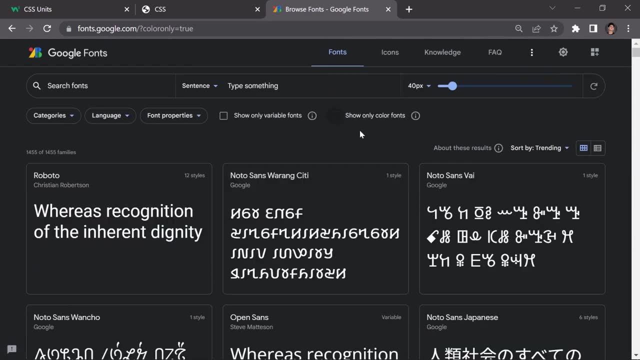 fonts. i've never used this one before. okay, so it will just allow you to just provide a color for kind of uh, emojis and stuff. you can play around with that if you want to. you can increase or decrease the font size. if you want to, you can even change the text. let me just write something. 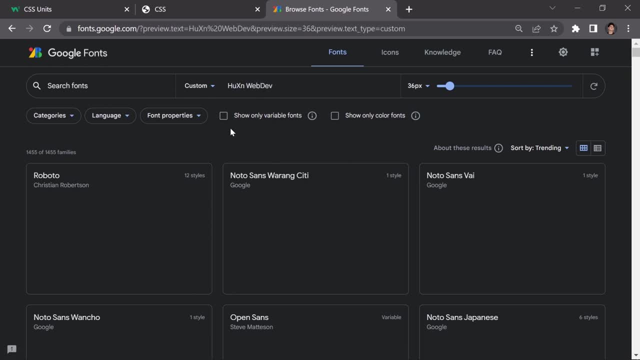 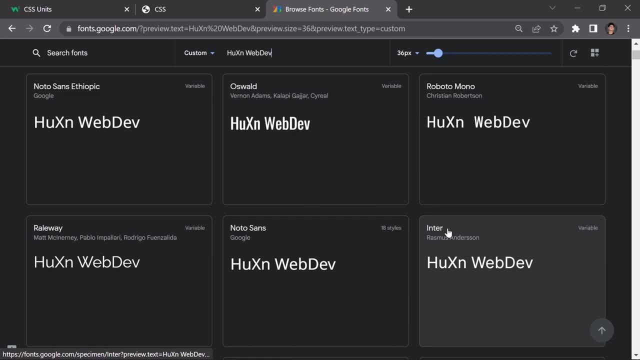 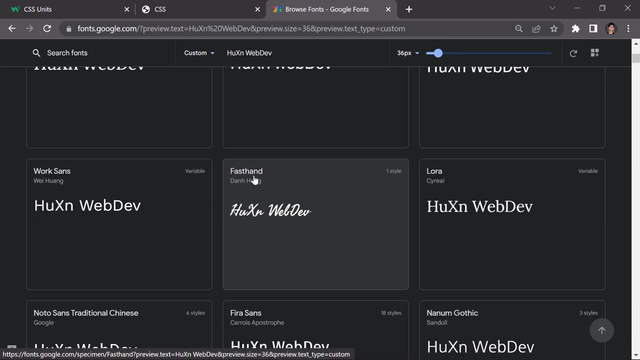 else like my own name: huzzain web dev. okay, so here you can see to allow change all of the text to this huzzain web dev, and now i can see it clearly right here. okay, so suppose if i want to get this one as well, so i want to get some crazy one like this one- uh, i can't pronounce the name of it, but 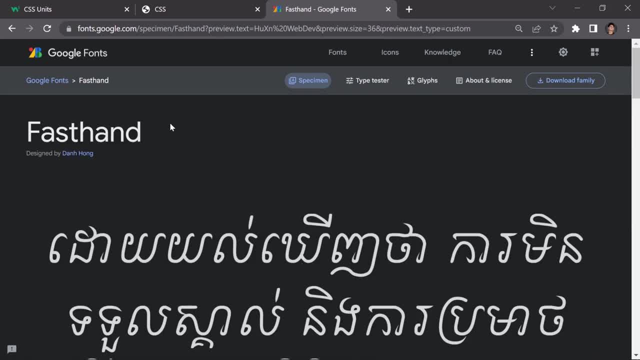 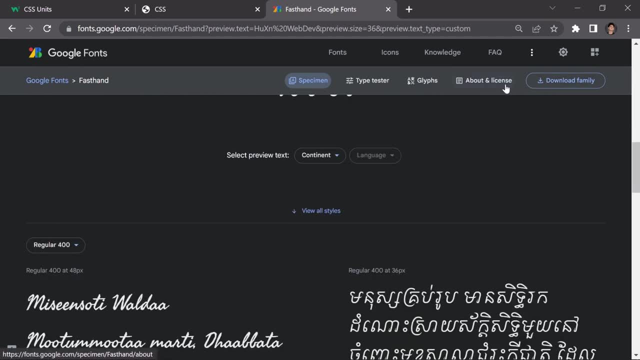 if i click on that, so it will now brings us to this font page right here. okay, don't be scared of this gibberish. you can download this font by just clicking on this font family, but you don't have to do that for now. so if you just click on there, then select all of the font which is inside that. 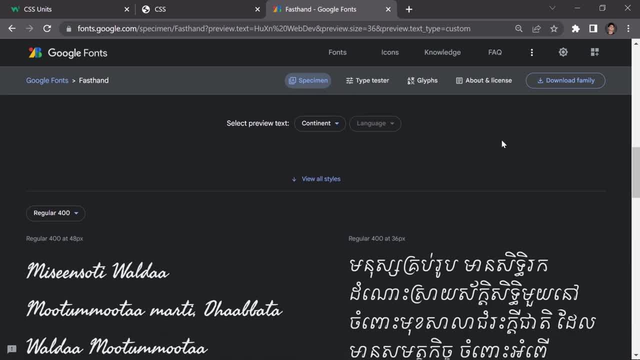 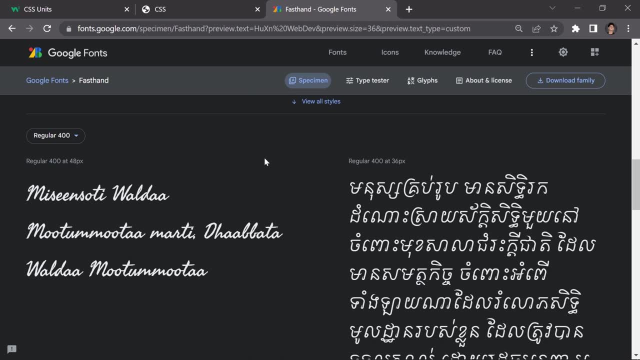 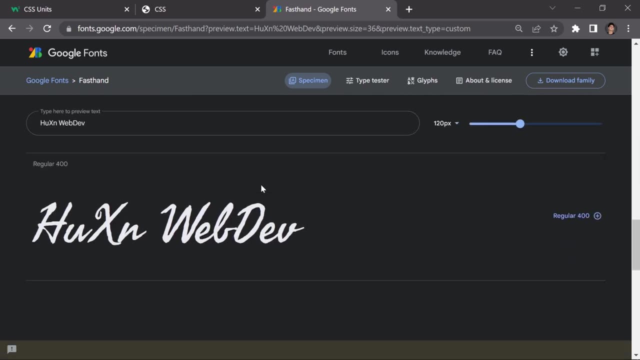 folder and then right click on it and click on install font. so we'll just install in your machine, but it will not work on the users machine. so if the user doesn't have that font, so it will not work on there. so if you want this font to send it to users, so for that what do we have to do? we have to first of all get into the 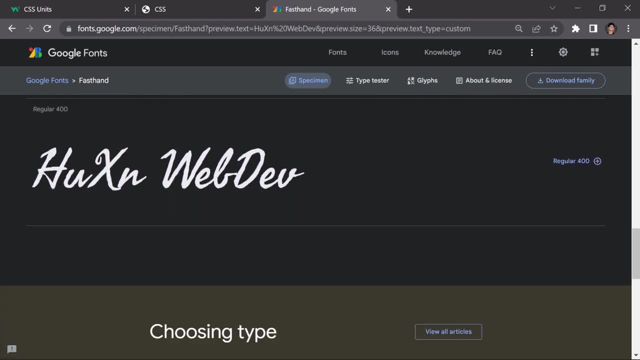 font and here you will find a lot of font weights right here. but for this specific font, this font just have, like this, regular font weight and if you click on that and it will now edit right here to this view, selected uh family, so if you click on that, so here you can see, it's already added. 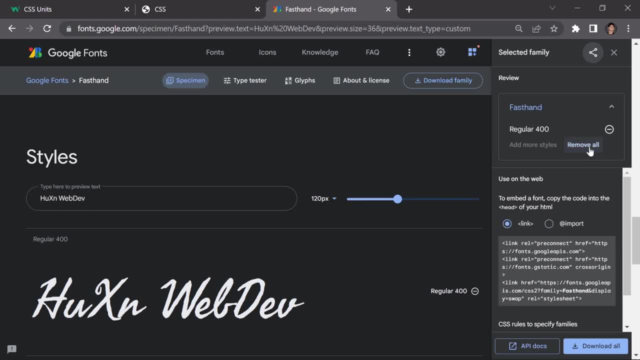 right here. if you want to remove that, you can just click on this remove all. or if you want to add more styles to so, you can just go back and add more. uh font families. if you want to, it will give you this link. you can put this link inside the head area, but i'll not recommend you to do that. 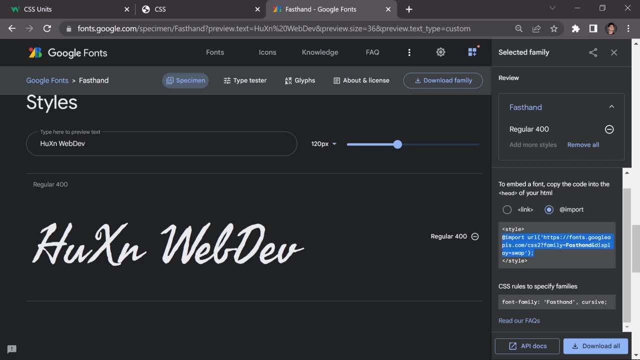 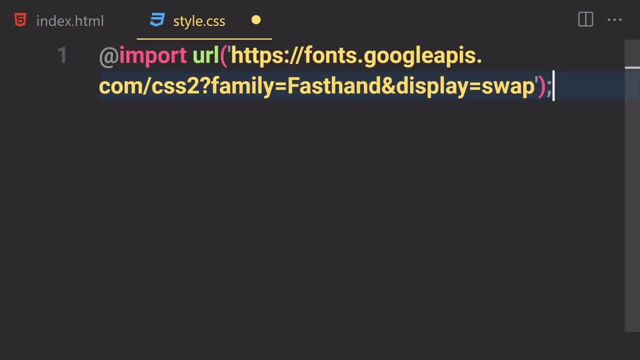 you can just click on this import and then copy this import, not this style opening and closing tag, but i want you to just right click on it then copy it. so once you copy that, then i want you to go to your style sheet right here and paste it right here somewhere inside the style sheet, right. 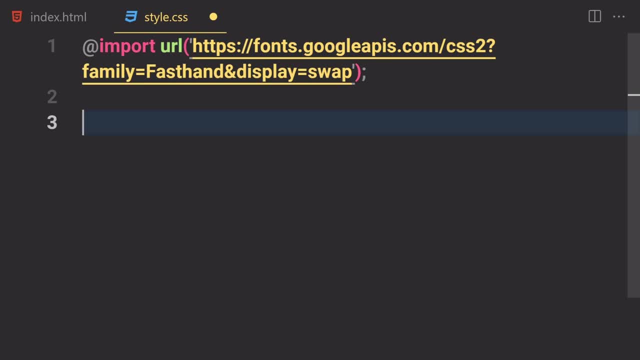 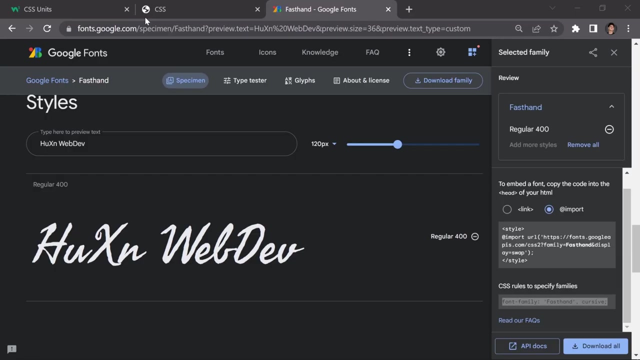 here. okay, it doesn't matter if you put it above or beneath, but the convention is to put it above. developer start working on your project so they can see the form family and stuff. okay, so now i'm going to just copy this font family from there. and now what do i have to do? i have to select this: h1. 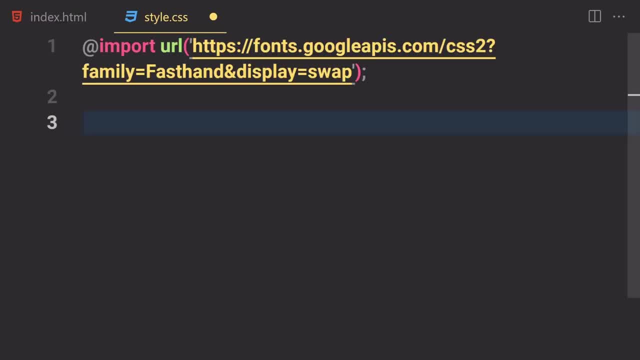 by default it looks like this: if i want to change that to this form which i selected, so i'm going to just write like a h1, and let me just write a form, and then family. and now here we can paste our own font, family, which we just copy from this area right here. okay, so now we paste that, right. 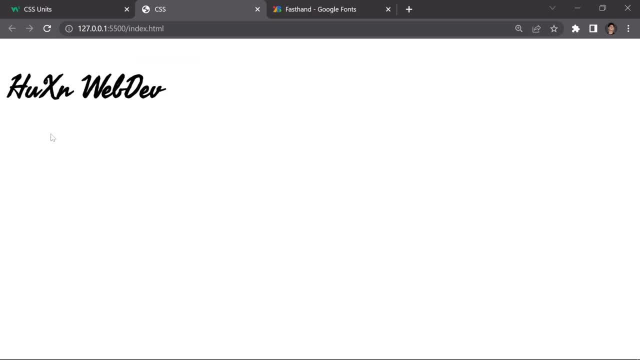 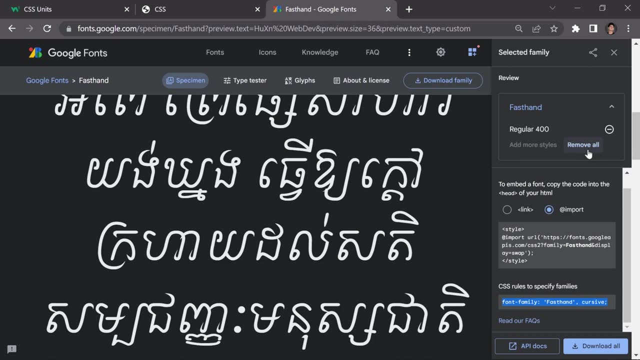 here. i'm going to remove this column as well. and now, if we save our file, and now here you can see, our phone will look like this right now. okay, so you can choose whichever kind of form family you like. so you can just remove there and you can choose whichever kind of form you like. there are. 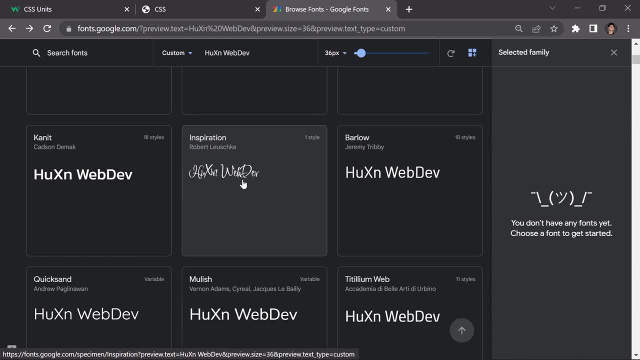 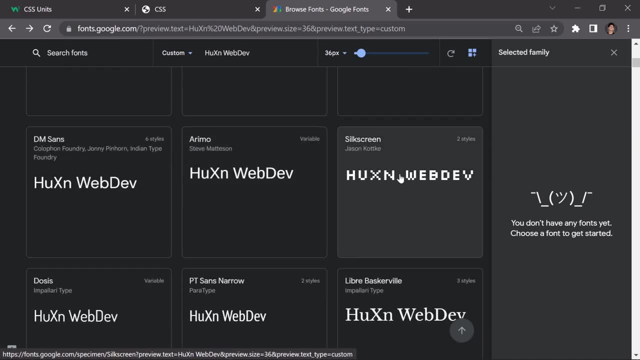 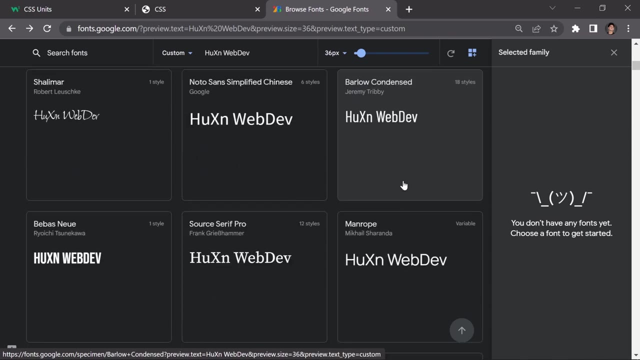 a lot of them like: look at this one, this is how my name will look- like kind of a logo and you can choose. like a lot of fonts, this one kind of a old-school game-ish, like a mario kind of font. there's a lot of them. if you want board, you can search for board. italic, uh, so on and so forth. 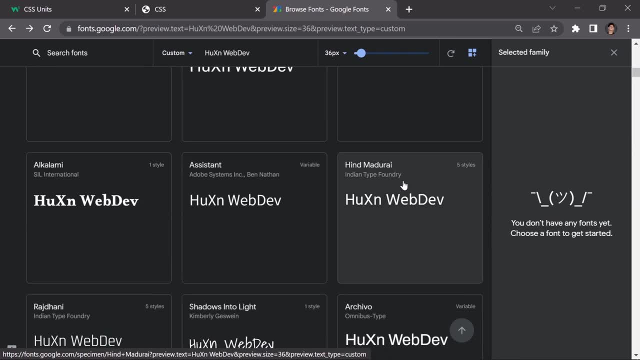 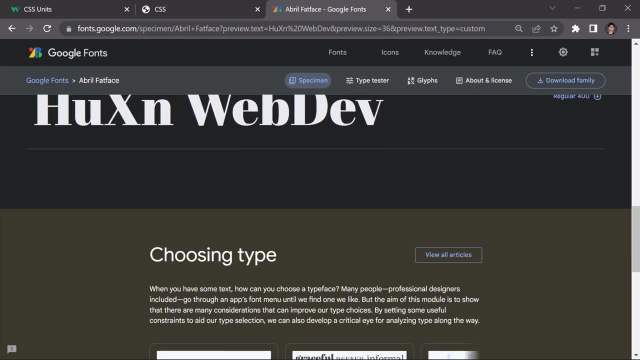 you know what i'm going to show you, the final font. if you want to get that for yourself and a real abriel kind of awesome font, let me just get that real quick and let's see: okay, this one also have one for family, come on. so i'm going to click on this. 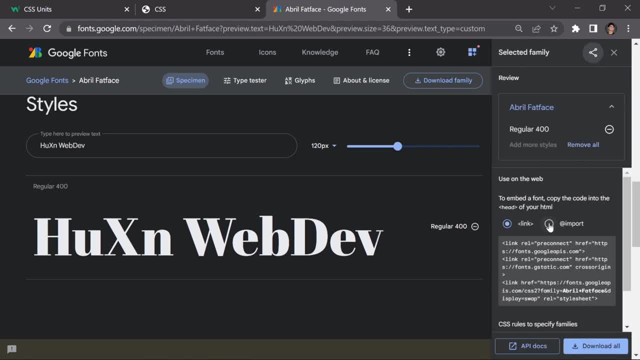 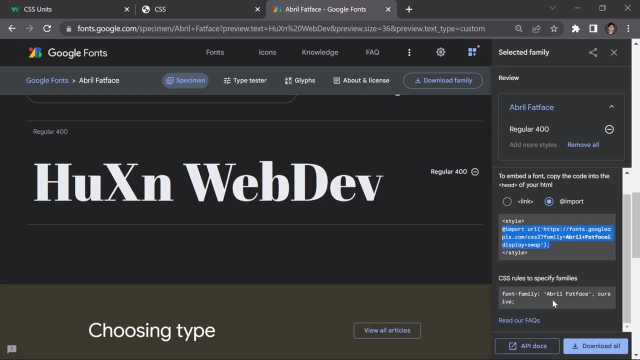 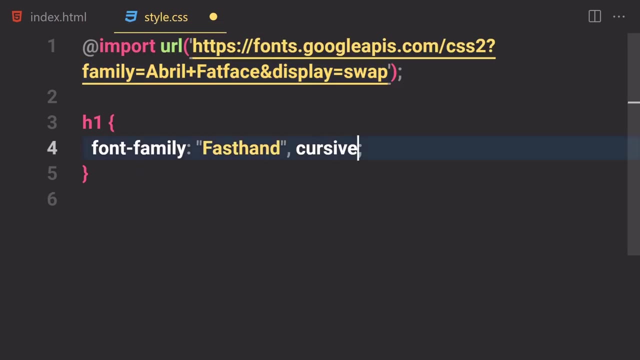 one. it will add it right here. so now i'm going to click on this import, i'm going to copy that and now i'm going to remove this one and replace it with this new font, and i'm going to copy this font family from here and i'm going to be pasting it right here. come on. so if i just paste right, 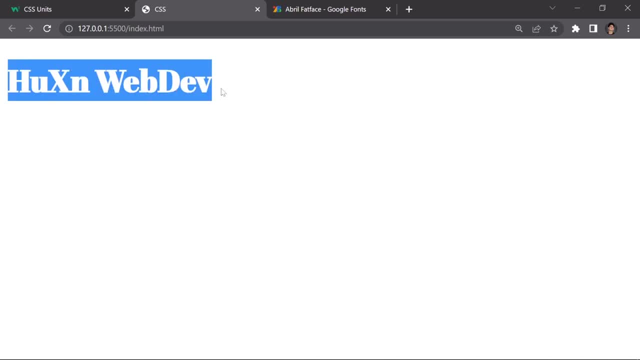 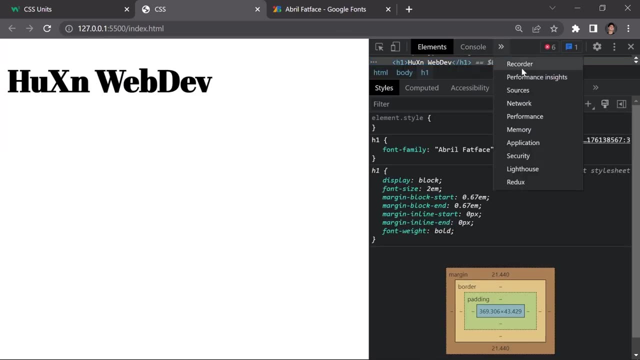 here and if you save our file, so now here you can see this how our phone will look like right now. okay, so if you right click on it and go inspect, and then we have to go to uh net for panel, and now, if i just refresh that, and now here you can sit and load down on this. 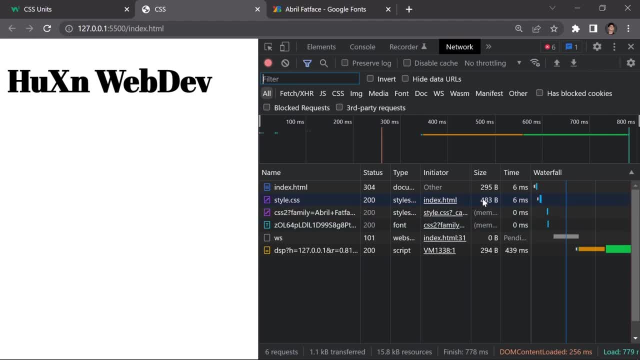 phone. and how much is this phone? okay, it's not that much huge. so we have like 483 bytes of font. okay, so this is our style sheet. this is our style sheet. where is our phone? all right, so here you can see. we have our phone. if you click on there, you don't have to go to the details. i. 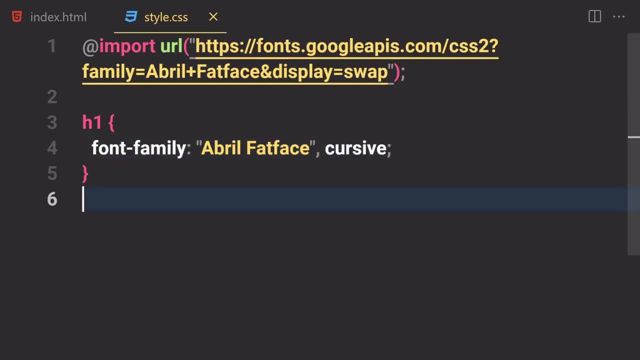 don't want to show you their details, but you know, you know that how to render a form and stuff you, so now we are totally done with the topography section. now the next section i want to talk to you about is a box model. so we are going to be learning about padding margin content. 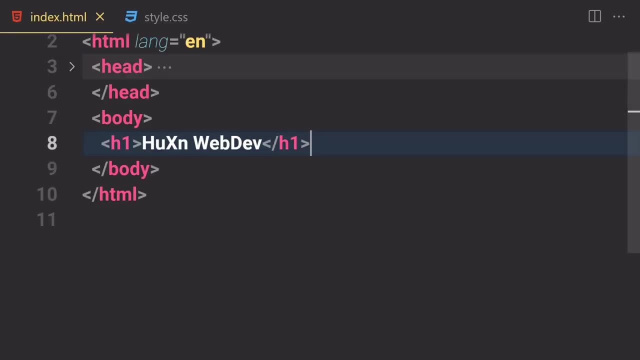 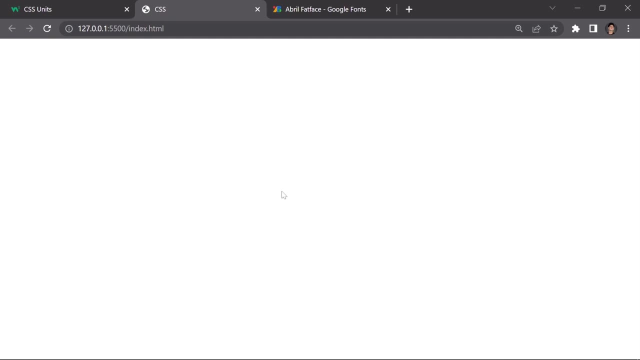 and border and stuff. so i'm going to remove everything from here and everything from the body as well. so here you can see, we have a clear body right here. so now, what is a box model? you don't have to go to the details of it, but everything on the web is made up of a box. 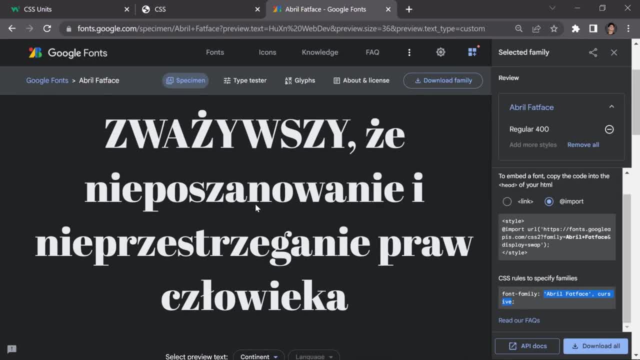 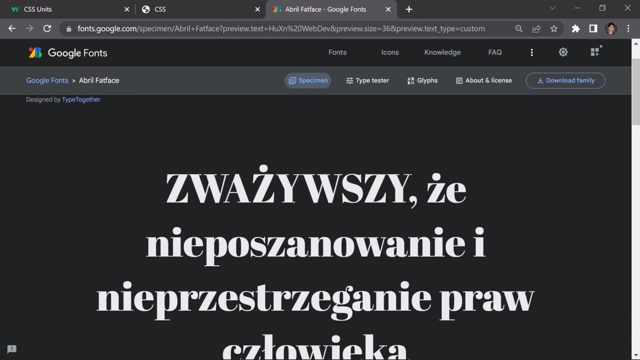 so what do i mean by that? if you go to any site like, it doesn't matter which kind of site you're, which kind of site you want to visit, you can visit to any site. so everything you see on that site will be made up of a box. what do i mean by that? if you click on this one, this one will be. 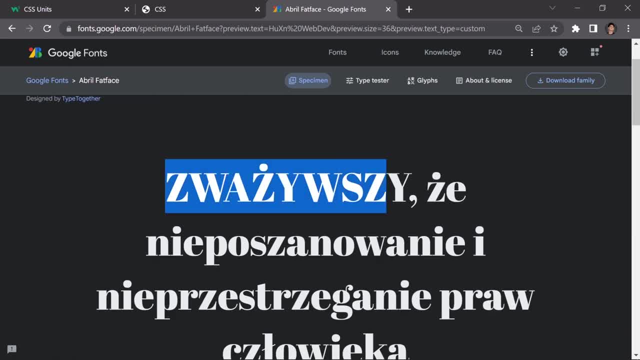 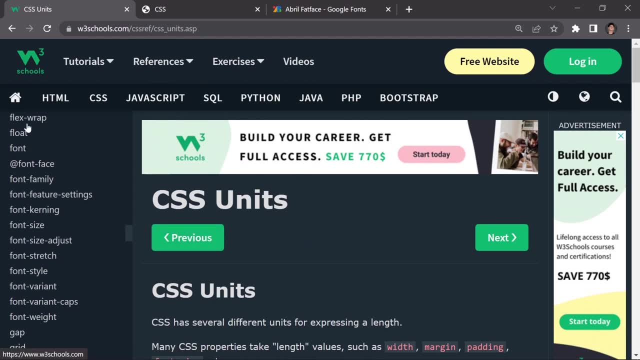 a box. this one will be a box. this one will be a box. everything you see like this will be a box. these will be a box. if you go to a css, so all of them will be our boxes. this will be a box. everything is a box. so if you just right click on it and go to the inspect area right here, 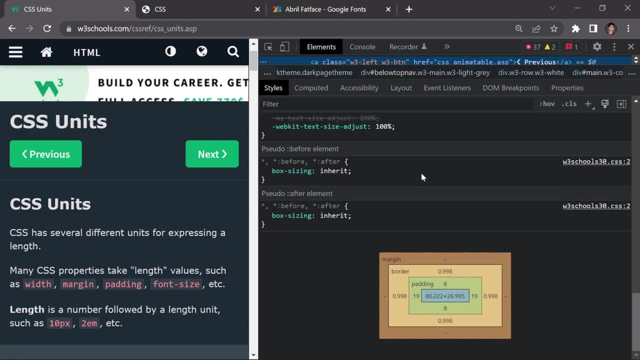 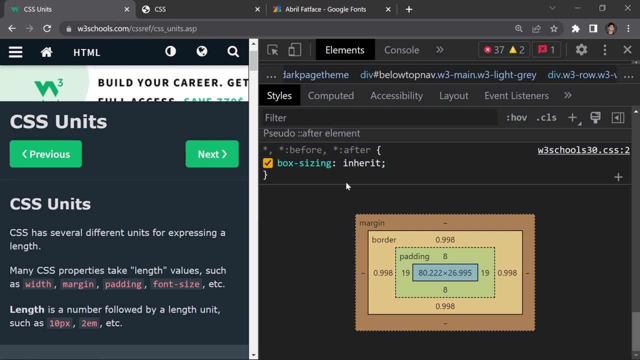 so if you just scroll down, scroll down, so what do we get? we get this box, kind of a shape right here, kind of a box right here. so what is inside this box? everything on the web is made up of a box, and their box is made up of four things. so which kind of four things? i'm 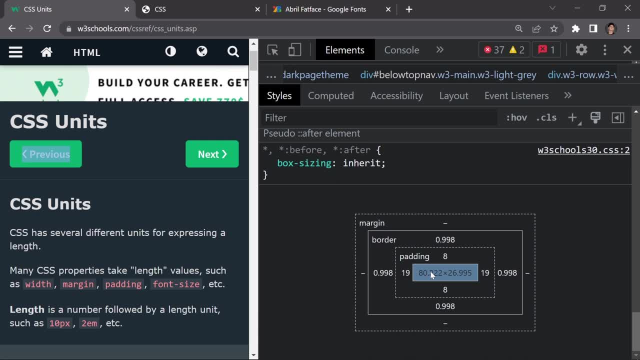 talking about. the box is made up of a content- this is the first one, then we have a padding, this is the second one, then we have a border- this is the third one, and then we have a margin, and margin is the fourth one. okay, so you just have to remember that. let me just say that one more time. 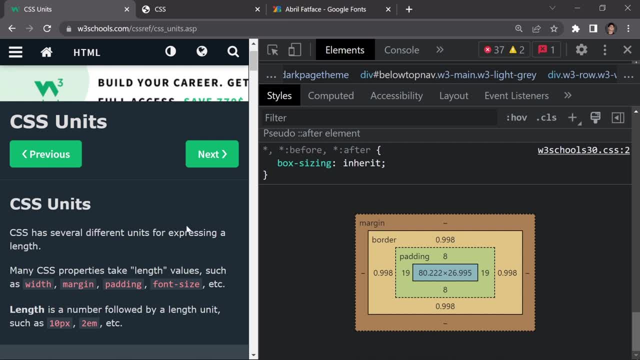 everything on the web is made up of a box and that box is made of content, padding, border and margin. okay, so if you want to provide a margin to this button, so you can also do that by writing here like i don't know, 200 pixel and here you can see it will not provide. 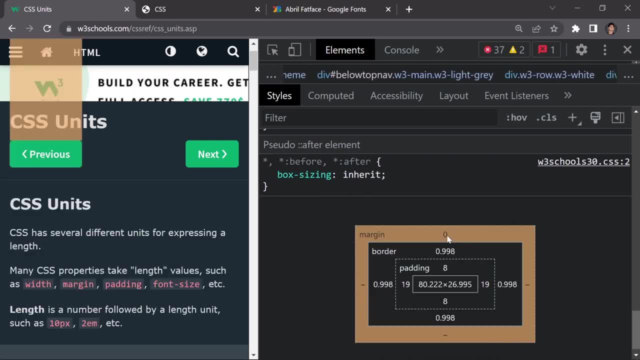 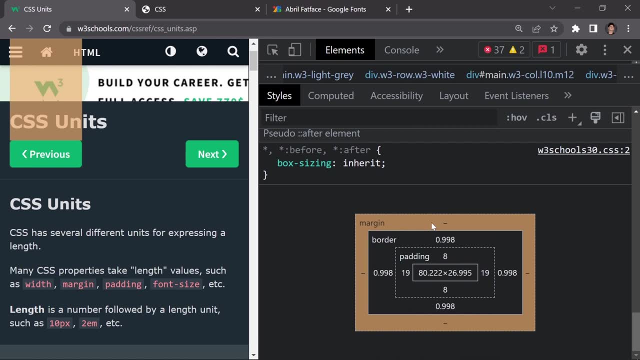 that margin. you don't have to worry about everything for now, which i'm doing inside this box model, but you just have to sit back and relax and watch it. okay, so now we can change the content area, if you want to. we can change the padding like, let's suppose, for top and bottom. it's awesome, but 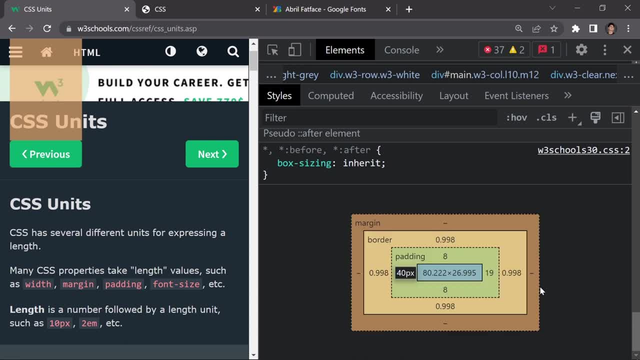 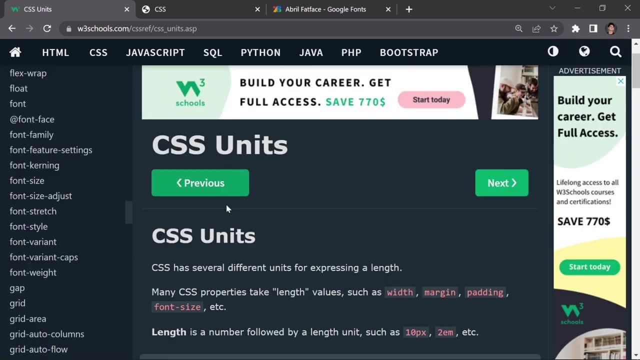 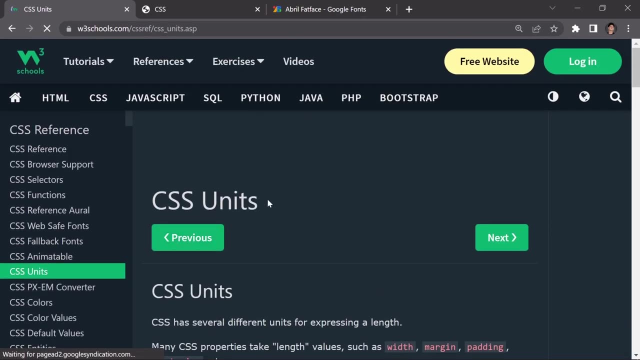 if you want to change the padding, if you're not sure and you don't know how to do so, then if you want to change it, there's some other options, like here. you can show the size. let's just say that this is what i'm going to write inside the button, so i'm going to create. 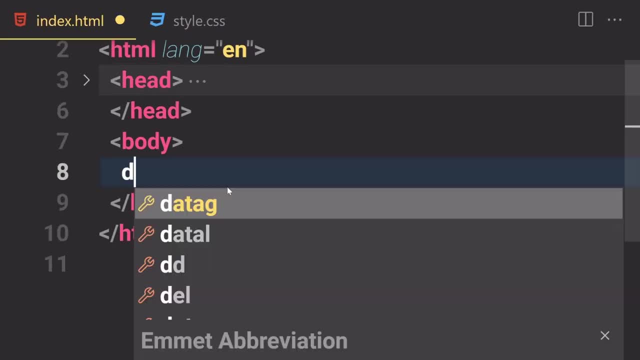 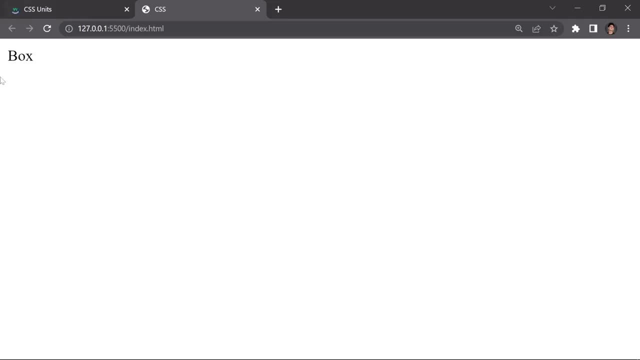 a selection on the left and right. i'm going to do is that i'm going to just provide like 40 pixels div in here and i'm gonna write nothing at all. you know what? i'm gonna write a box box. so if you save that and now here you can see, we have a box right here. okay, so if you want to style this box, 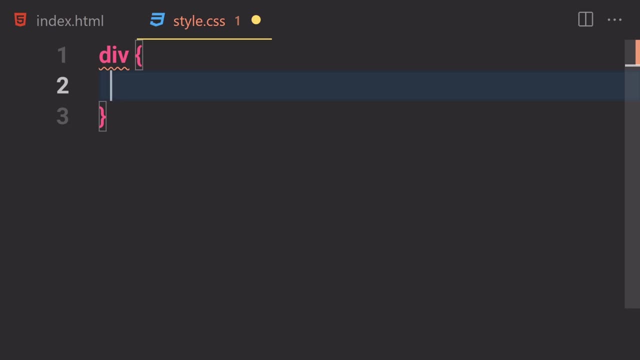 first of all, let me just get this box. then what i'm going to do is that, first of all, we are going to be learning about a border. so, in box model, first of all, we are going to be learning about a border. so, if you want to provide a border to this entire area, like to in this entire box? so 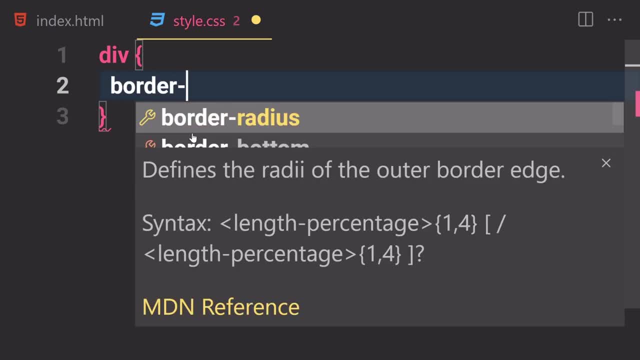 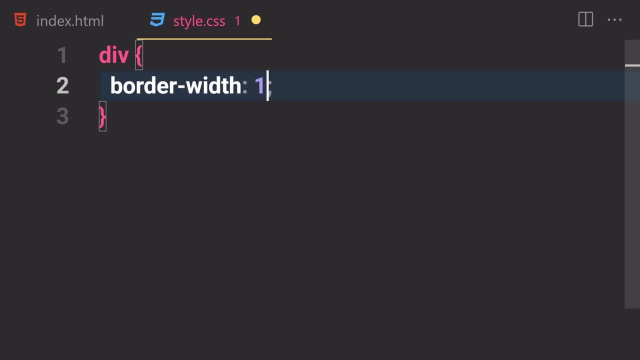 what do we have to do? we have to just write a first of all the border with, like how much will be the width of our border? so we can just specify the amount, like in my case: uh, we can write one pixel, we can write two pixel, 100 pixel or how many you like, but in my case i'm not going to. 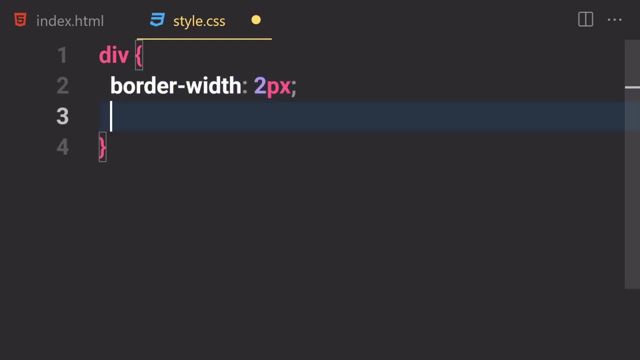 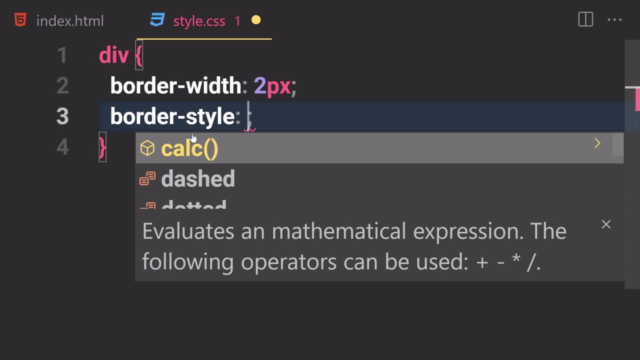 go that much crazy. i'm going to just write like two pixel of border width. then what else do we have to do? we have to just write a border and then style, and so what will be the style of our border? so we have a lot of kind of different styles. we have a dash dotted grew hidden. 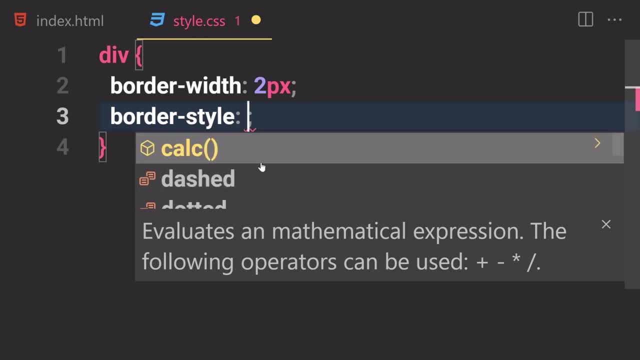 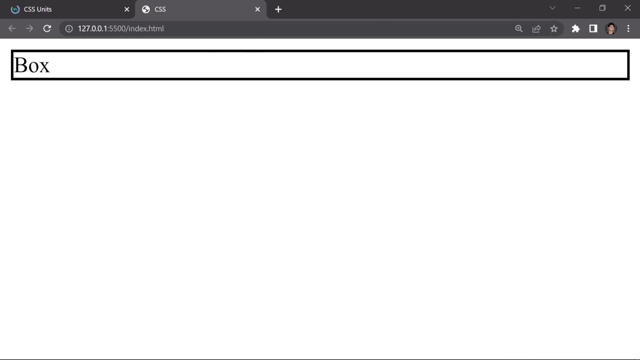 and so on and so forth. and now, in this case, what i'll do is that i'll just write like a solid one right here. okay, so now, if you save file, so what do we get? we get this border right here, around this box, right here, and if you right, click on it and go to inspect area. 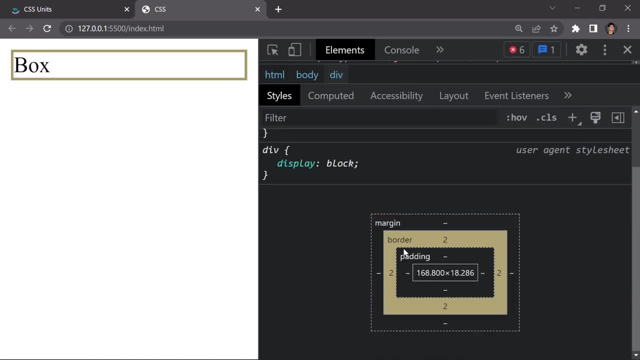 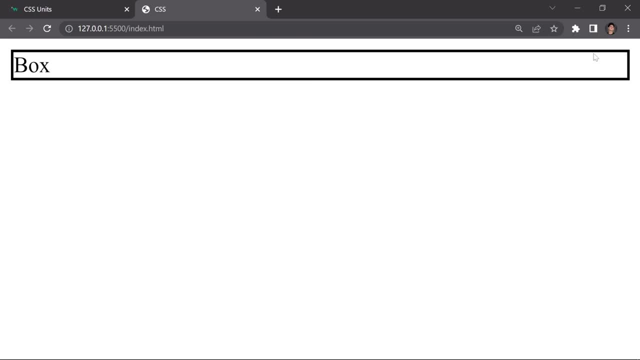 and now, here you can see, we have this border all around this area, right here. so we have border to the top, border to the bottom, border to the left, border to the right, and so on and so forth. okay, so now we get our border. so now, in some cases, we would need to change this. 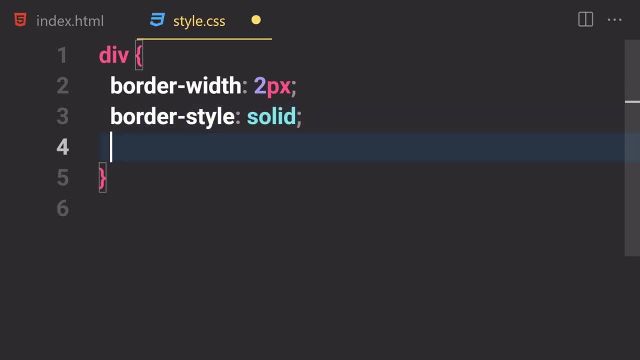 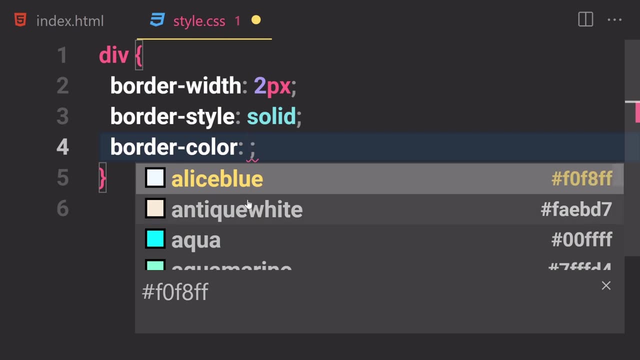 border color. so if you want to change the border color, so for that we can just write like a border and then color. okay, so it allows us to change the border color to be like any color as you like. you can provide rgb value, you can provide hexadecimal value, you can provide hsl, you can provide rgba. 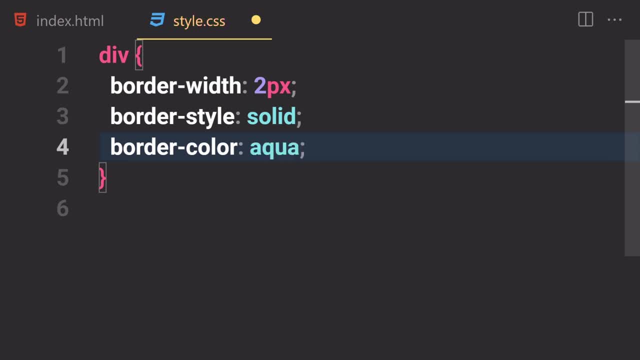 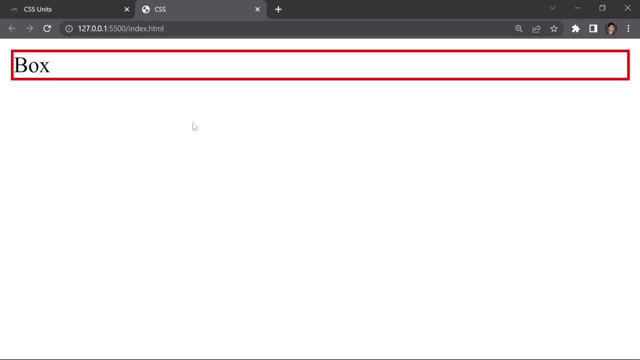 value if you want to, but in my case i'm going to just click on this aqua one and now, if you save that, and here you can see, it will not change this color to acquire. you know what? i'm going to just stick to red and save it. so now, here you can see, change. the color is changed to red, right here. 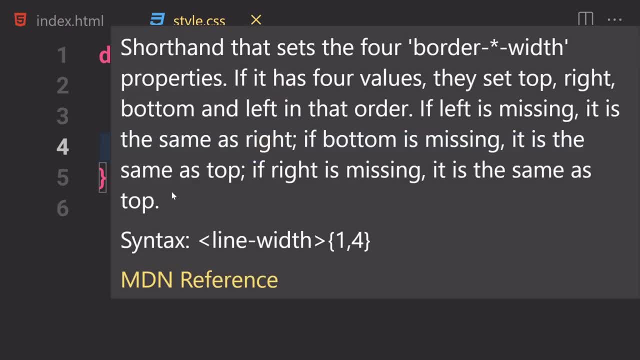 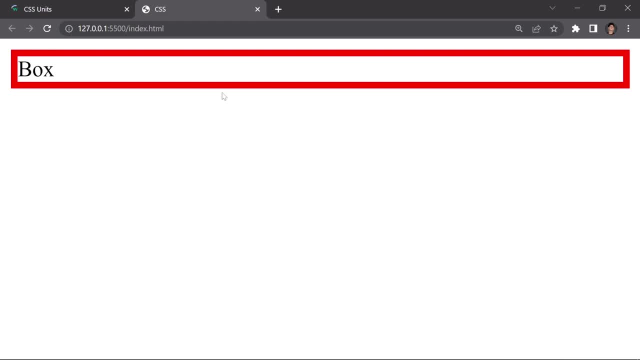 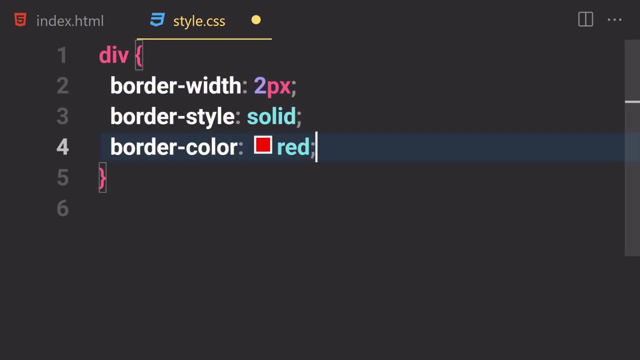 okay, you can increase or decrease the size of this border by just specifying it right here, like: uh, maybe, uh, five pixel borders to save that, and this is how you can provide a border to it. okay, so this is the long way to write your border. so now let me just show you the shortcut for writing. 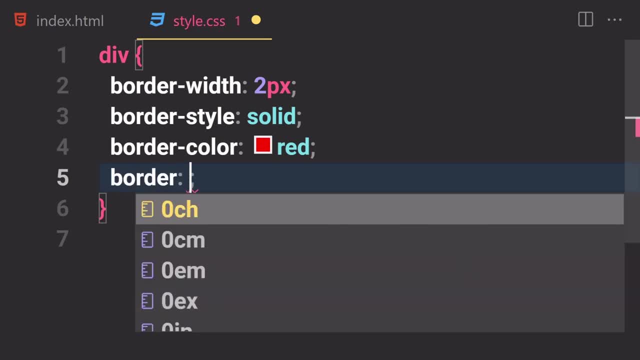 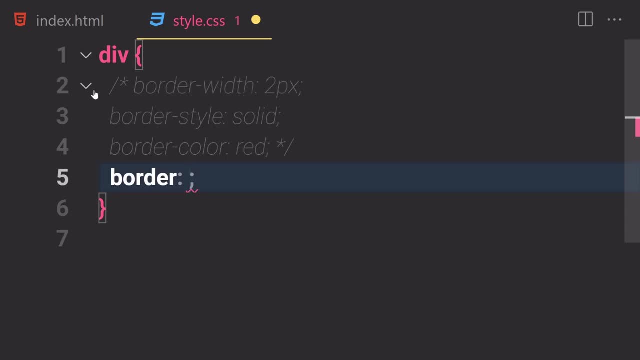 a border. so what do we have to do? we just have to write a border right here. so so now i'm going to select everything and i'm going to comment all of them out, and now the first parameter or the first value we are going to be providing is the border width. 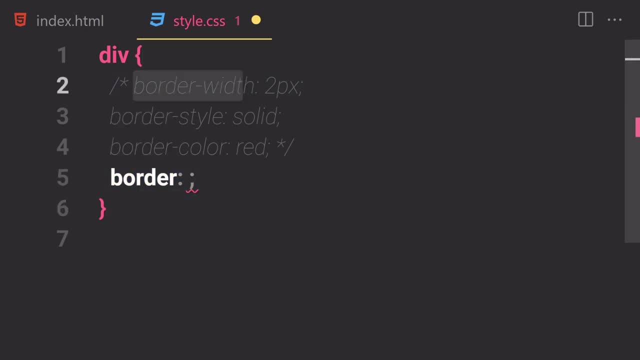 width, like we are going to be providing first of all the border width property, then the border style property and then the border color property- uh values to be precise. so first of all i'm going to just write like two pixel for the border width, then i'm going to just write like uh, in this case. 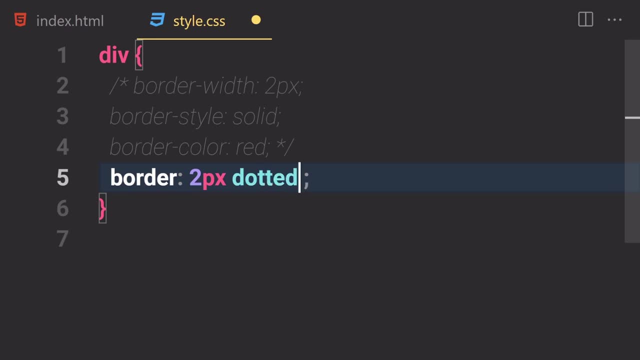 i'm going to just stick to like a dotted one. so i'm going to select a dotted kind of border and then, finally, i'm going to provide a color to be like, maybe teal color. okay, so this is the shorthand for writing a border. so now, if we save that- and now here you can see, the color is now changed to. 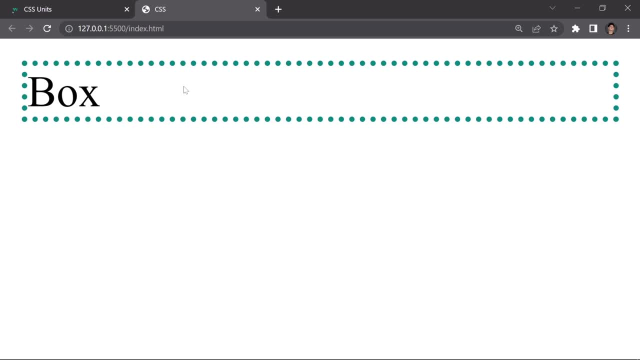 teal, the style is changed to this dotted one and now we have this border all around it, okay, and we have two pixel kind of a border. we can increase or decrease that, like 10 pixel maybe. now here you can see that border become a little bit bigger. okay, so you can play around with that if you want. 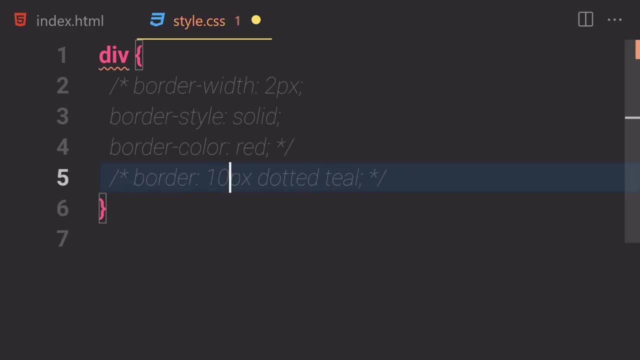 to. but now, if you want to provide a border to just a specific side, like in some cases, you just need a border for the top or for the left or for the right. so what do you have to do? you can just write like border in some cases, like you just write for a left, so left border. 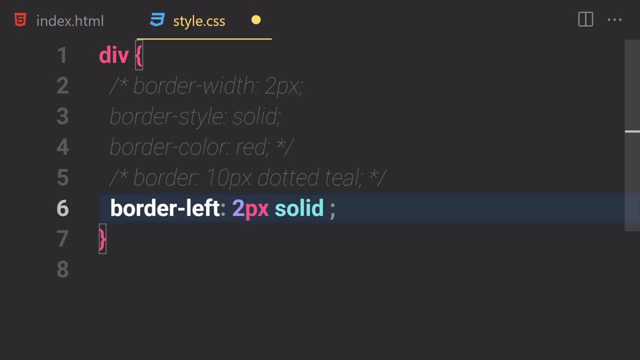 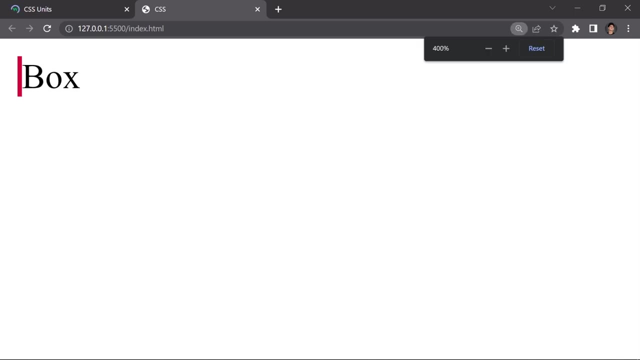 will be just like, uh, two pixels solid and then teal maybe, or maybe which kind of color you like. in my case, i'm going to just stick to the crimson and cell file. and now, here you can see, we have border to the left, if you want to push that to the right. so what do we have to do? i'm going to just 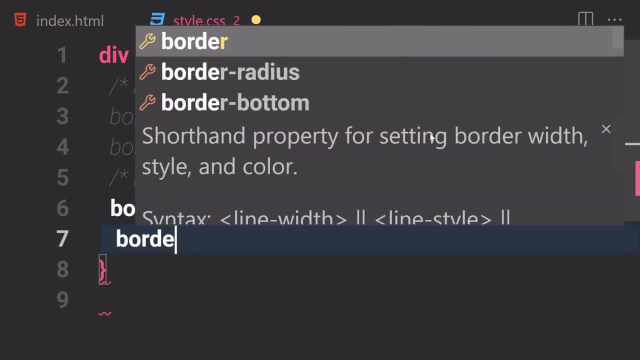 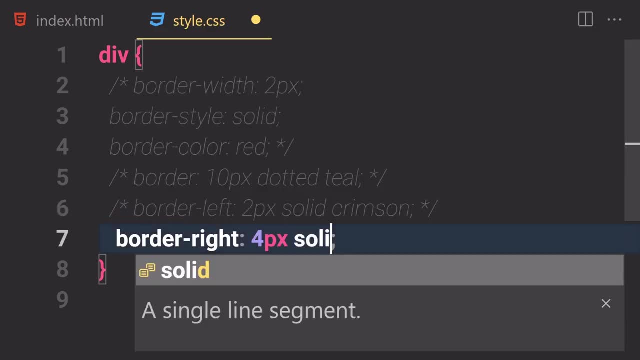 write like a border order, come on, border to the right. and i'm going to come in this line out and here what i'll do: i'll just write like, maybe four pixels solid, uh, of um, kind of uh, which kind of color you want to use? maybe i'm going to just click on this blue violet. i'm going to have to. 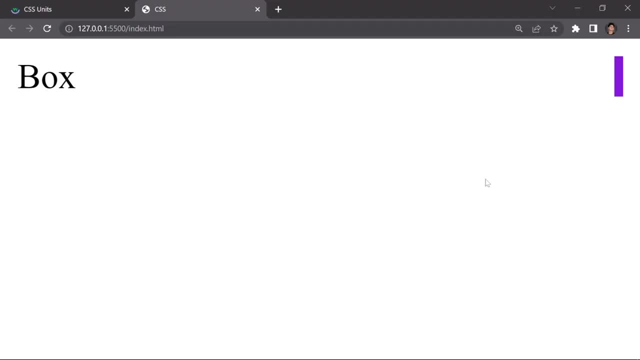 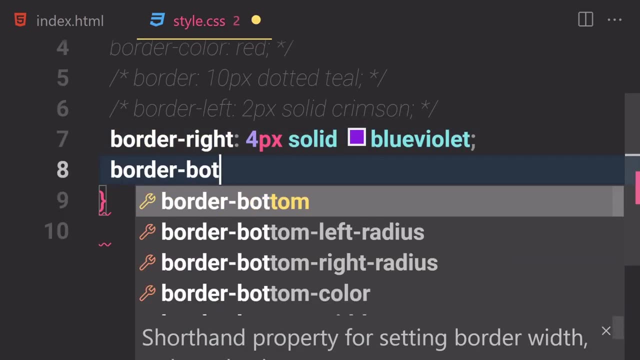 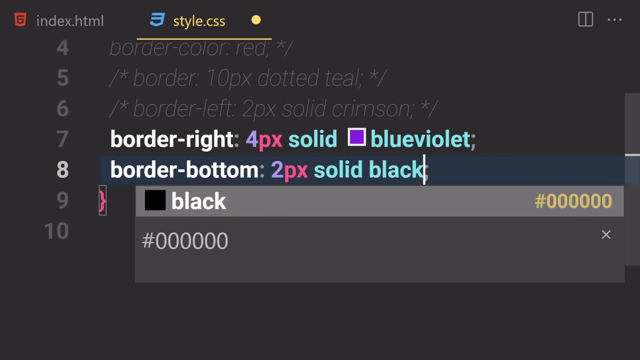 write it manually like blue, violet color. now, if you save that now, here you can see, we get our border to the right. if you want to get it for the bottom, so we can just write like border bottom and we can just write like two pixels solid off. uh, maybe, uh, which kind of color would be fine? black, 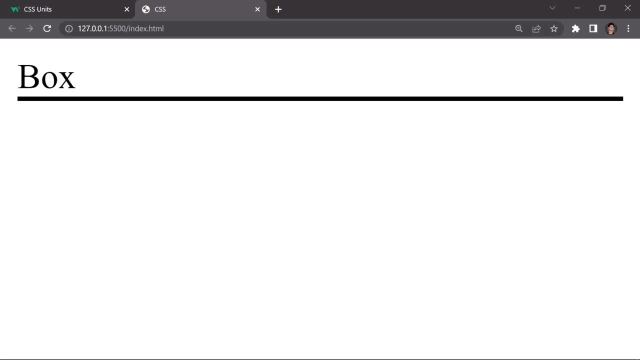 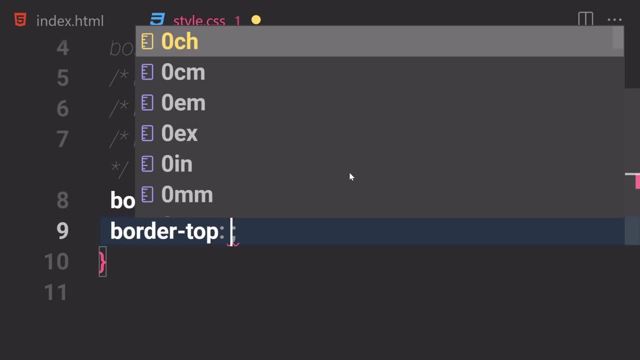 would be fine. and i'm going to just comment this line out and if you save that now, here you can see, we'll not just add the border to just a bottom. if you want to put it for the top and bottom, you top, so we can just write like border top of two pixels solid or whatever, like teal maybe, or 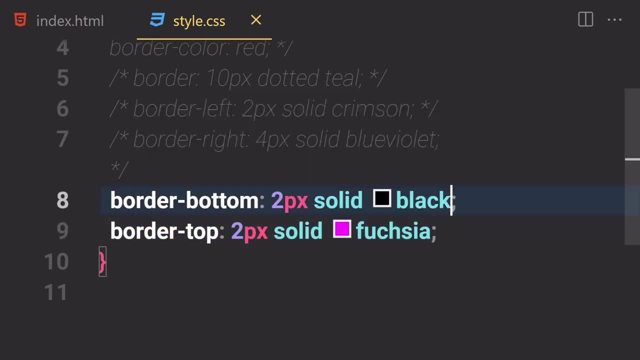 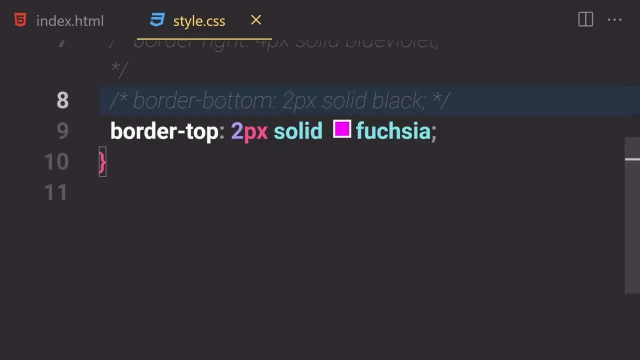 crimson or fuchsia. so i'm going to just select this fuchsia, come in the other one and here you can see it will add this border just to the top area right here, if you want to add it, for like all of the area one by one. so you can also do that. if you want to, i'm going to come in this. 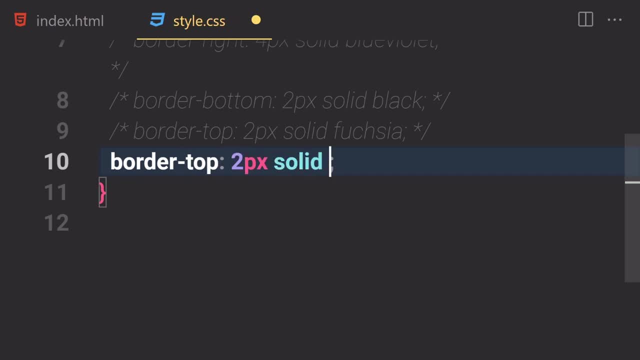 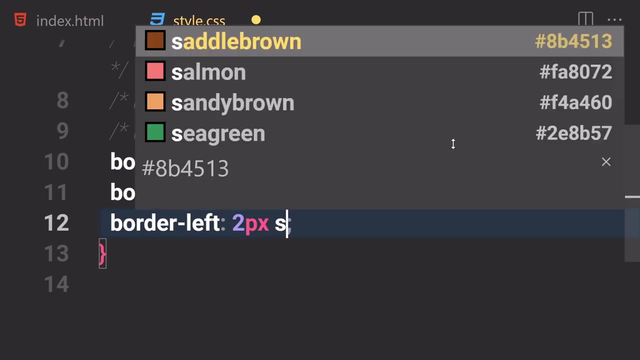 one. so i'm going to write like a border to the top, first of all, with two pixels solid- uh orange. then we have a border- uh, come on. border to the bottom of two pixels solid- uh what teal. then we have a border to the left. you would just get like two pixels solid of green. then we have a border. 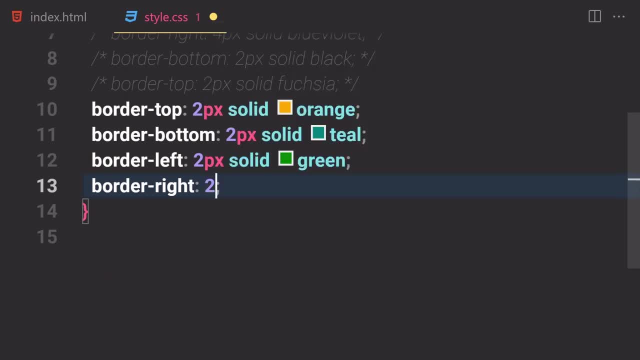 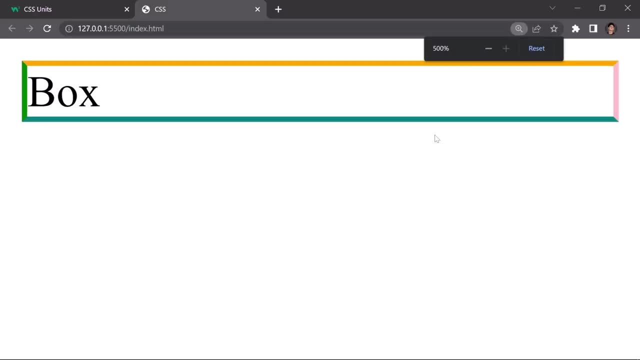 to the right- i'm going to zoom out of it- or right, to be like two pixels solid and maybe, i don't know, pink would be fine. and now, if you save that and here you can see, it will now add this border to all of this area and we have different kind of colors for it. 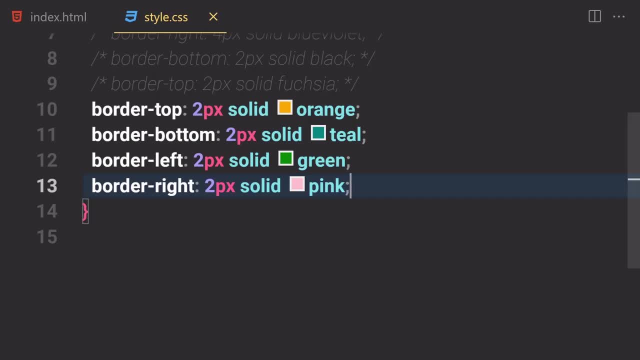 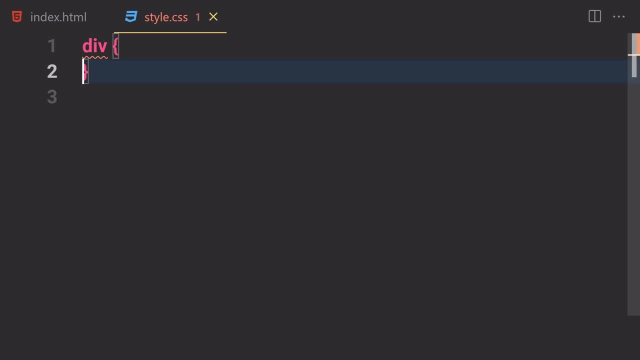 okay, so this is how you can add a border. so what i'm going to do is that i'm going to remove everything from here, like so, and zoom it over, and now here i'm going to just provide a specific border, like two pixels solid of red would be fine, and now, if you save that, and now there we go. okay, so now we learn. 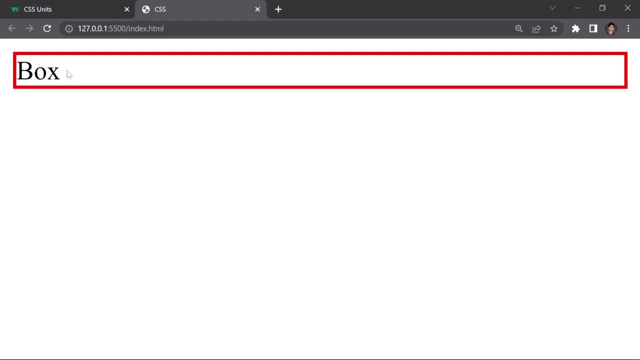 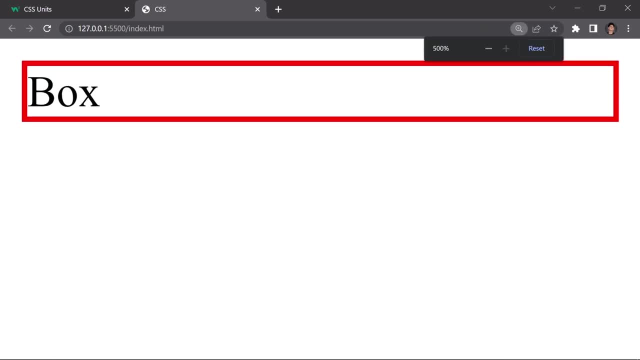 about how to add a borders to a specific kind of box or container, whatever you want to call it. now let's just learn about something called padding. so what is a border padding? a padding will be just an inner space inside this box or container or box or whatever. 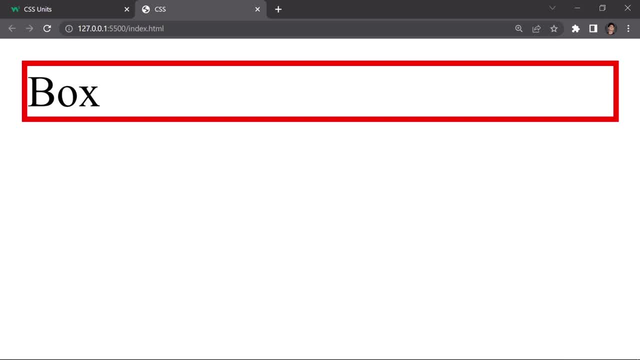 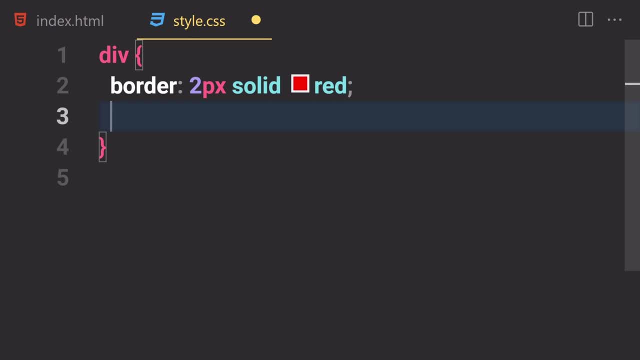 you want to call it okay. so we are going to be adding a padding inside. a padding is just an inner space of that container. so if you want to add this padding, so we just have to write like padding: first of all padding and then this is a shorthand for writing a padding. so i'm going to 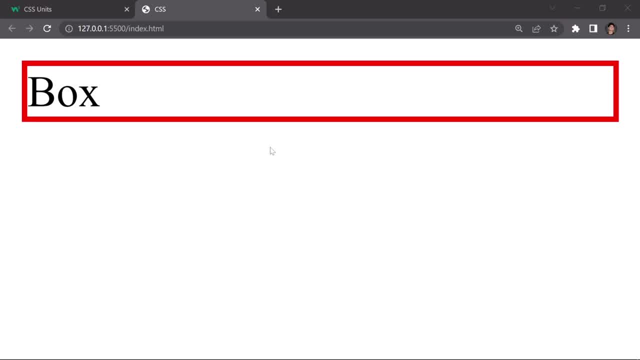 just write like 20 pixel of padding to all around. so if you save that and here you can see, we get like padding to the left, padding to the right, and then we're going to add a padding to the left, padding to the top and to the bottom, if you right click on it and go to inspect area and here you can. 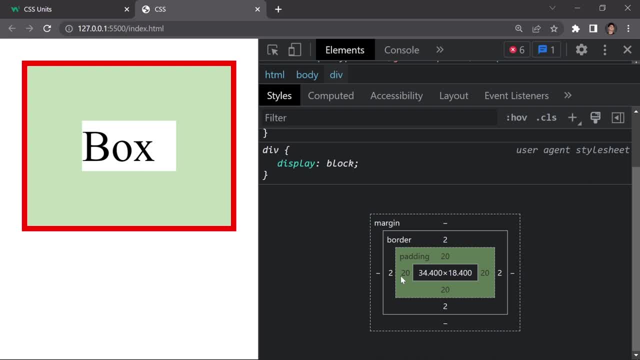 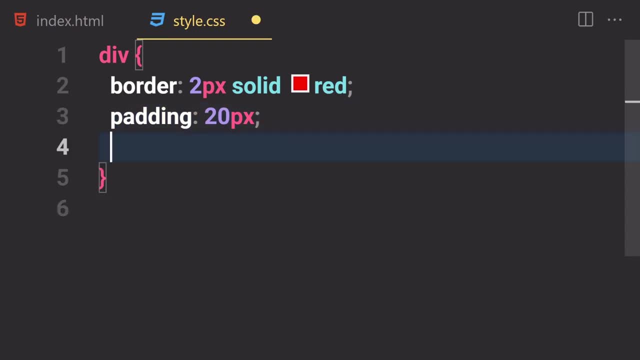 see, we have a padding to the top, bottom, left and right, right here and we also have this border to all of that area. so if you want to add it to a specific area, so all of that the same stuff will apply to this one as well. so we just have right padding to the top of 20 pixel and save our file. 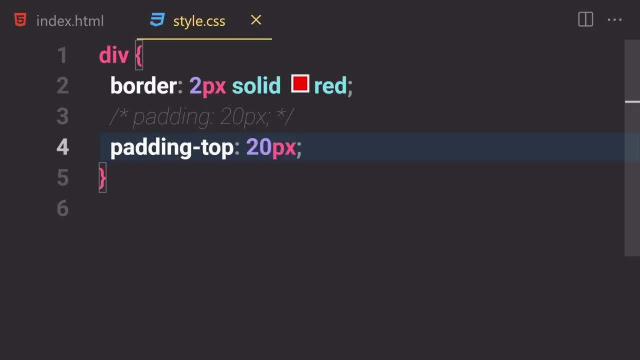 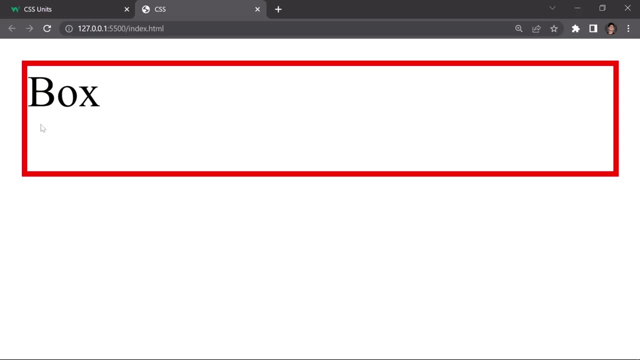 so it will now just add padding to the top, if you want to add it for the bottom. so you can also do that by just writing padding bottom of 20 pixel and then you can add padding to the bottom of 20 pixel and save our file. so we'll now just add this padding to the bottom if you want to add it for. 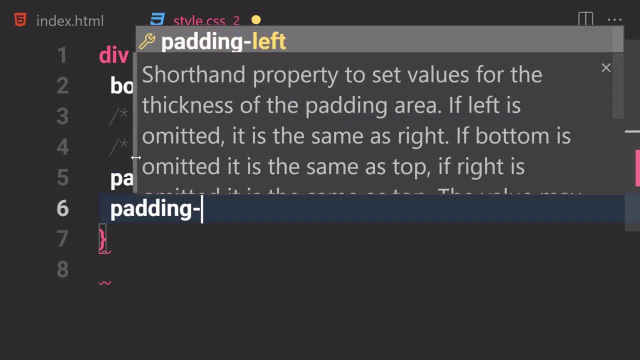 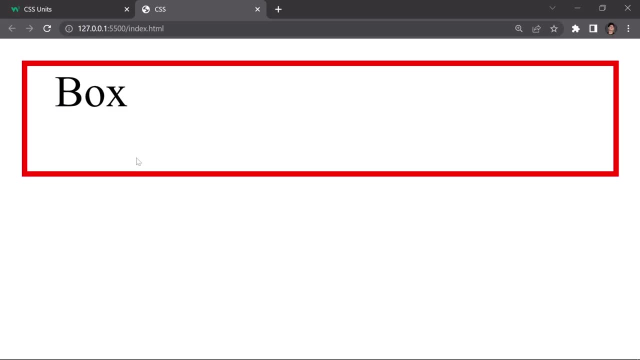 a left. so we are going to be writing like a padding of left and padding left, like in my case, i'm going to just write like 10 pixel and if we save our file and here you can see, it will now add this padding to this left area right here. okay, if you want to add it for the right. so before we're, 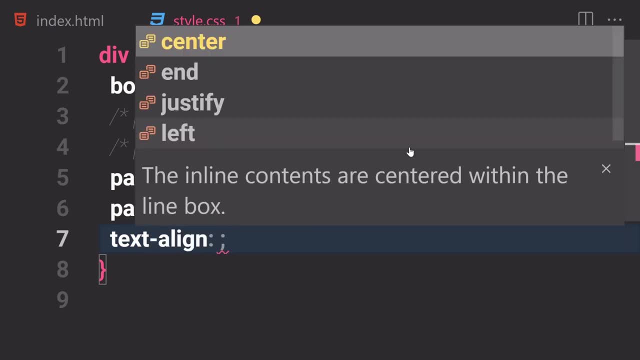 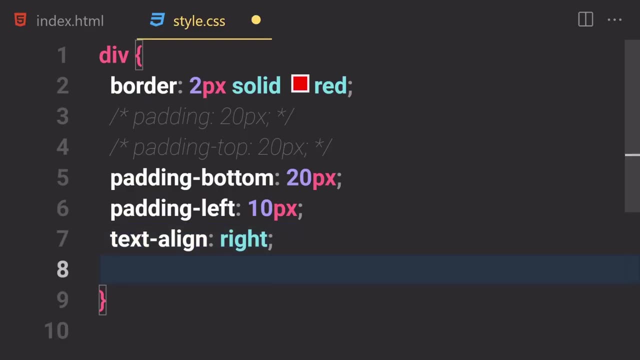 getting into that. we have to just write text align, as we learned a second ago, and text align to be the right. first of all, save it. and now, here you can see, we have this box right here and now. if you want to add padding to the right, so we can also do that by just writing padding right of. 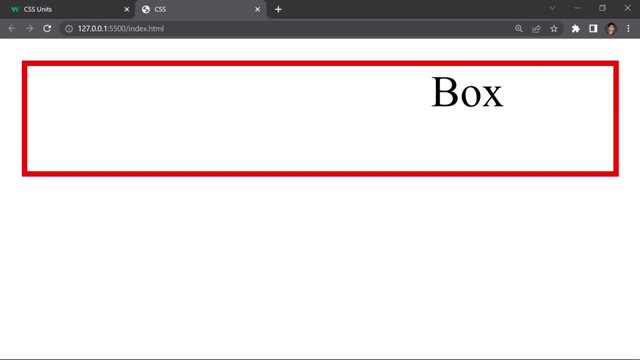 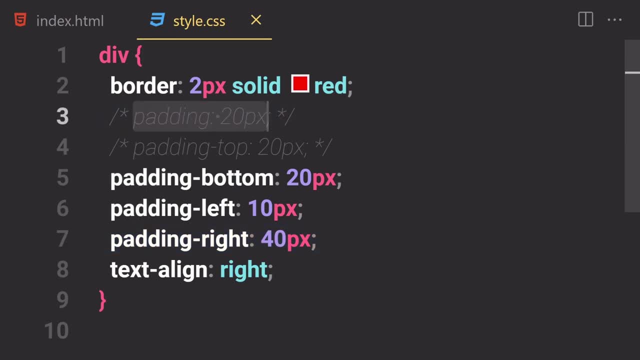 maybe 40 pixel. so if you save our file and boom, so you don't know, just add 40 pixel of padding right here if you want to edit all of the areas. so for that we have to just write like padding to the top, bottom and left and right. and now let me just show you one more uh, padding property which is like a. 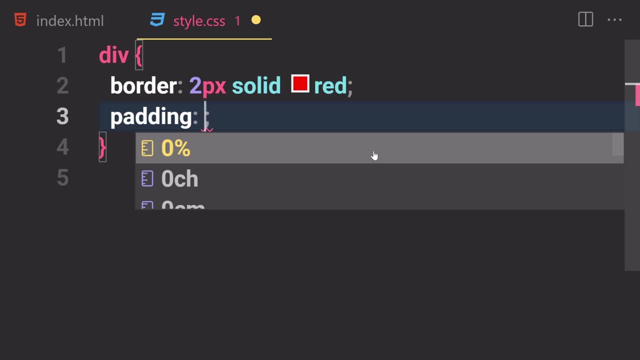 padding first of all. and if you want to add it for a top and bottom, so for that you can just provide like 10 pixel, and you don't want to edit for the left and right, so for that you can just provide a zero in here. so this is, the first value will be for top and bottom and the second value will be for 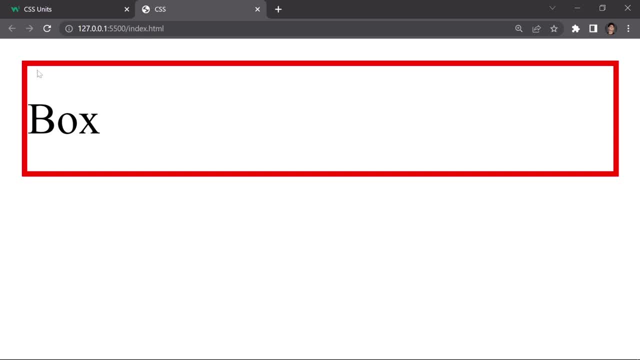 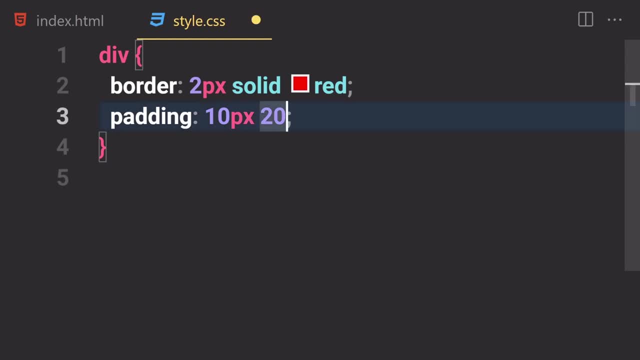 left and right. so if you save that- so here you can see- it will now add this padding to the top and to the bottom, but not to the left and to the right. so if you want to add to the left and right as well- so in my case I'm going to just write like 20 pixel, save our file. and now if you save there and boom. 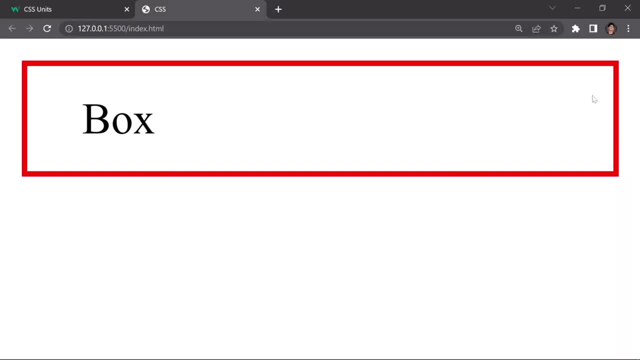 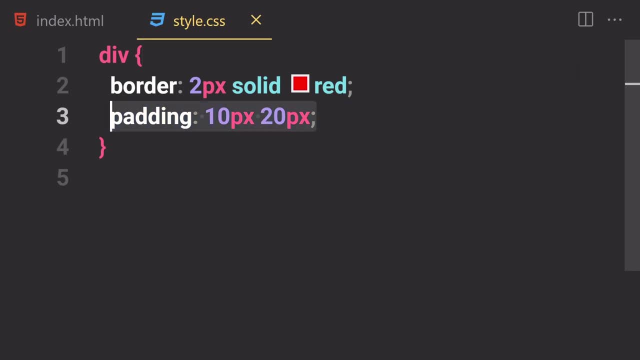 so here you can see, we have this padding to the left and you can also, you can see that right one, but we have uh also padding to the right one as well. anyway, uh, so that was it about a padding one. so now let's just learn about a margin, okay, so now we 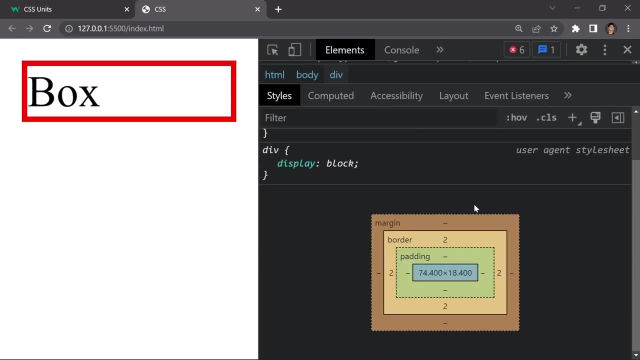 learned about these three things. so we just learned- or not three, but two things. we just learned about a border, we also learned about a padding, but we didn't learn about a margin. so margin as this one, like padding, was the inner space inside that container or their box, whatever. 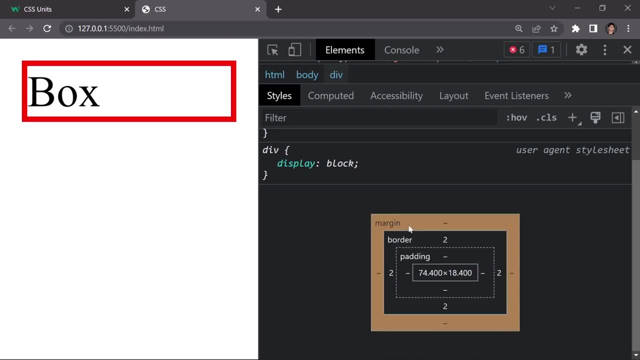 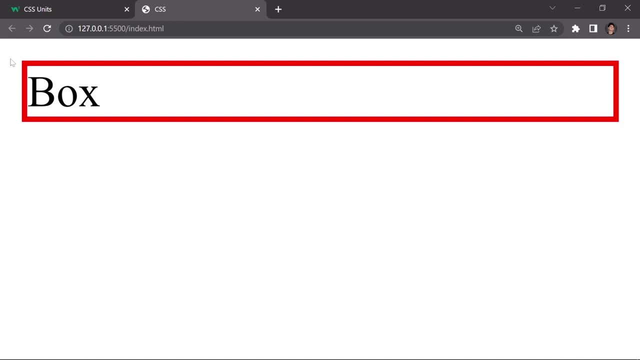 you want to call it, but now in this case their margin will be the outer space of that container. okay, so now if you want to add a margin and default here, you can see they added like margin to all of these areas right here, as i show in the 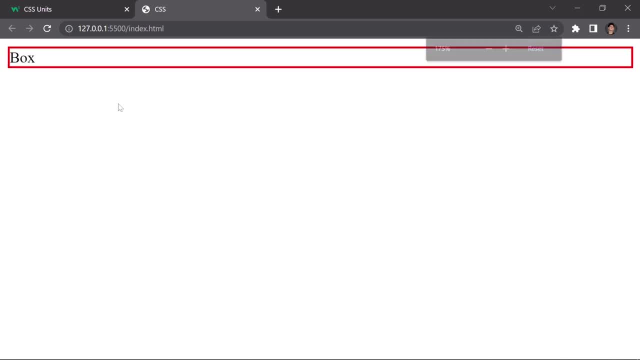 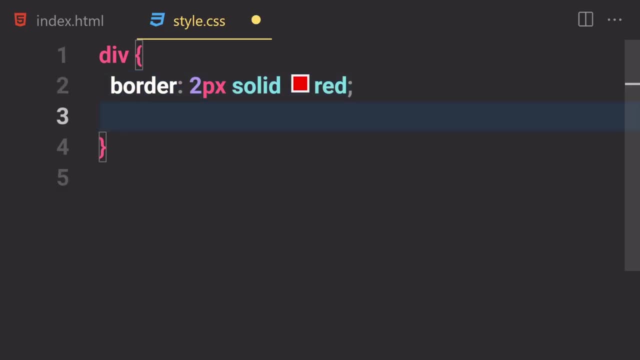 previous value. if you want to remove that. so you can just write like margin to zero. but now if you want to add a margin from to these areas, to a left and right and so on, so what do you have to do? you can just write like a margin and 20 pixel to all around. so if you just write that and if you save, 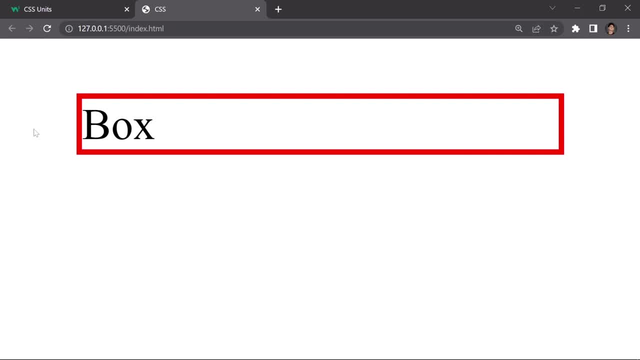 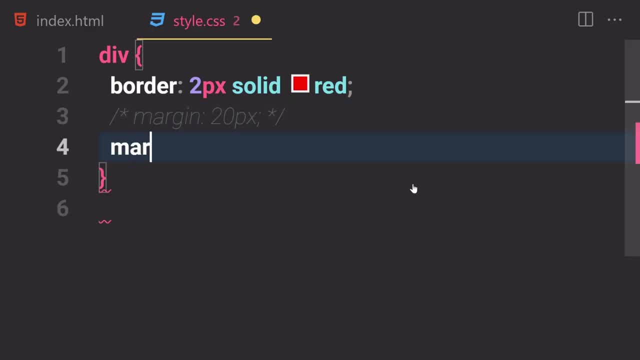 that. so it will now just add margin to all of these area, like 20 pixel to this area, top at top and bottom, left and right as well. okay, so if you want to add it to a specific area, so you can just write like margin of left and then 20 pixel margin uh right and 20 pixel margin uh top, and so on 20. 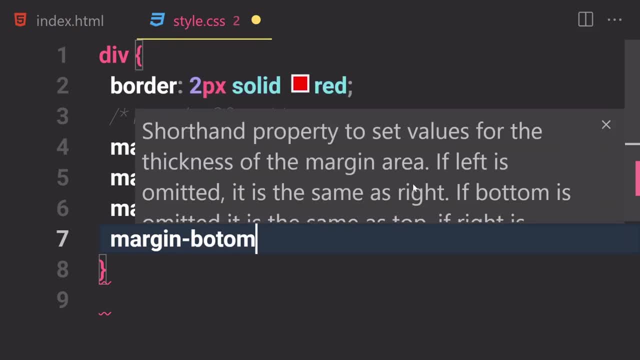 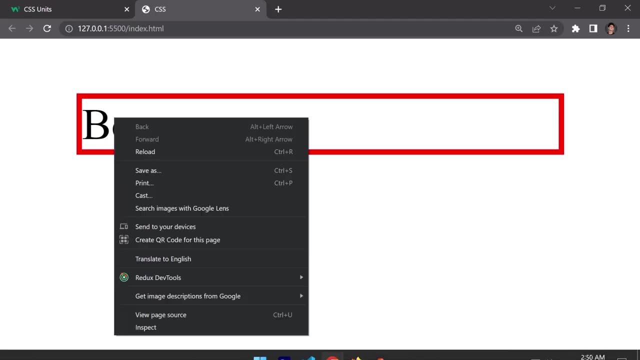 pixel margin: uh, top, bottom, and just write it for the bottom one as well, like 10 pixel, and if you save that and this is how it will look like right here and now, if you right click on it and click on this inspect area, and now here you can see, we have. 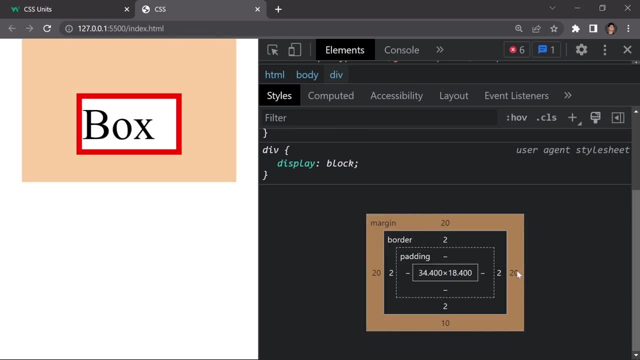 pedigree to the top of 20 pixel, left 20 pixel and right 20 pixel, and we also have 10 pixel to the bottom if you hover mouse over to the margin area, and this is how you can see there anyway. so we are now totally done with the box model, but we can also write like margin off, just if you write: 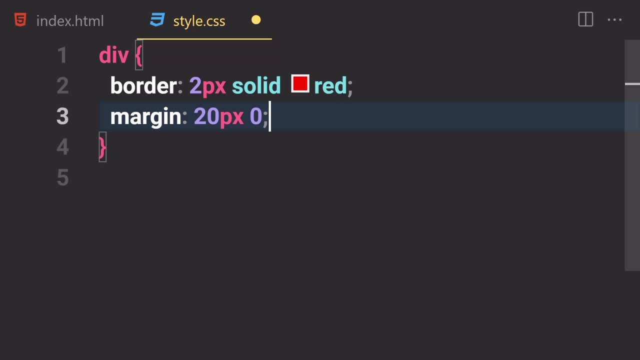 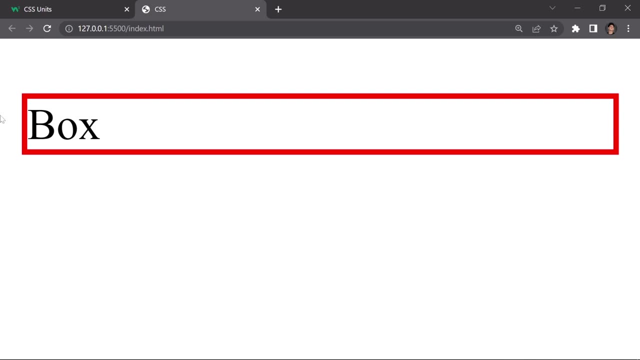 margin to the top and bottom, but not for the left and right. and if you save that, so we have margin for the top and for the bottom, but we don't have margin for the left and right. and now, if you are arguing like we do have a margin to the left and to the right and 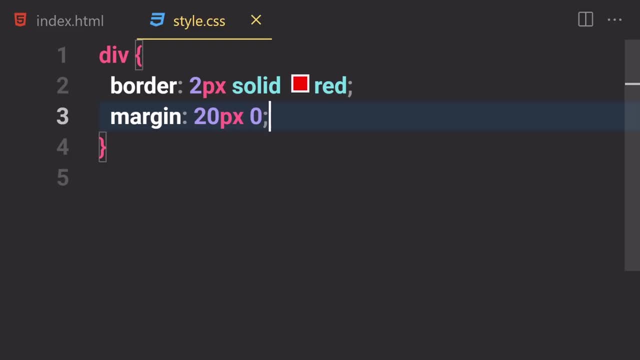 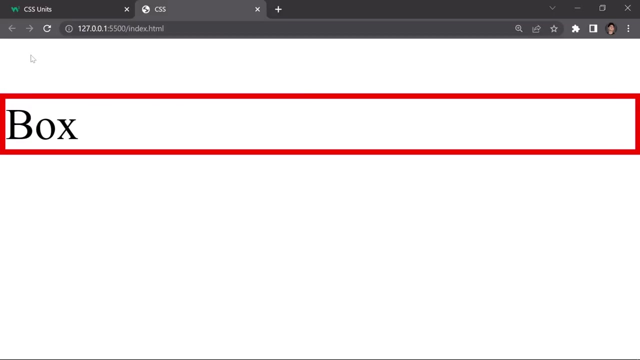 will just copy it and save from here. its saved, but I have nothing. BUT I don't have any margin. yeah, so we have margin from 20 pixel to the top and 20 pixel to the bottom, and we don't have that to the left and to the right. so if you want to provide there, we can set this one to zero, so we. 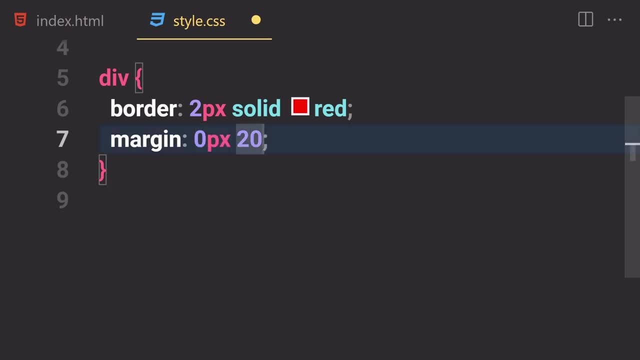 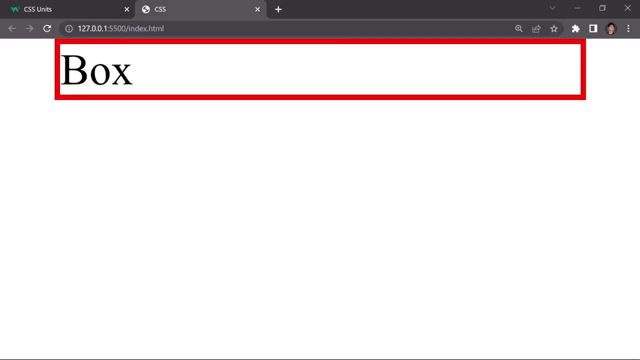 have top and bottom zero. but if you want to write it for the left and right, so you can just write 20 pixel. now, if you save that, and here you can see, it now gives the margin for the left and for the right of 20 pixel right here, okay. and if you want to edit for all of the area, so you just have to. 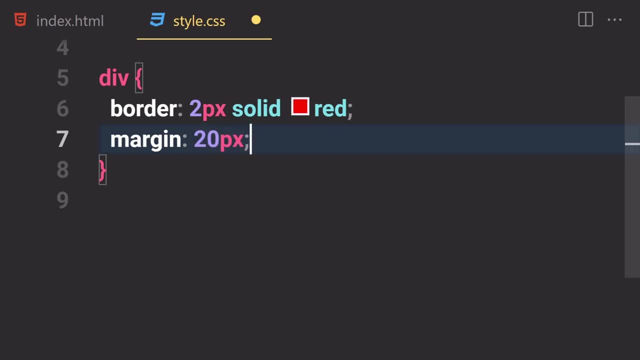 write margin of 20 pixel or thousand pixel, however you like, and boom, okay. so it will now add this margin to all of this area right here. so congratulations. now you totally understand a box model in css, and that was just a little bit of tricky and i will want you to play around with. 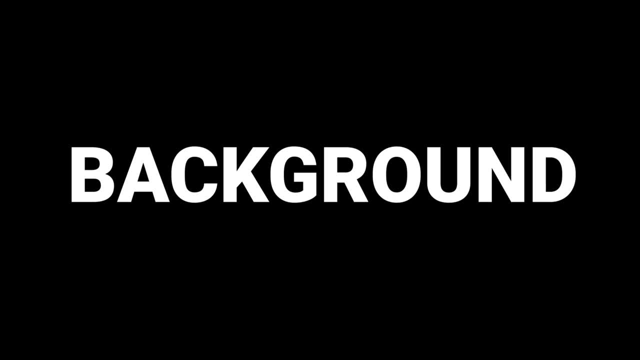 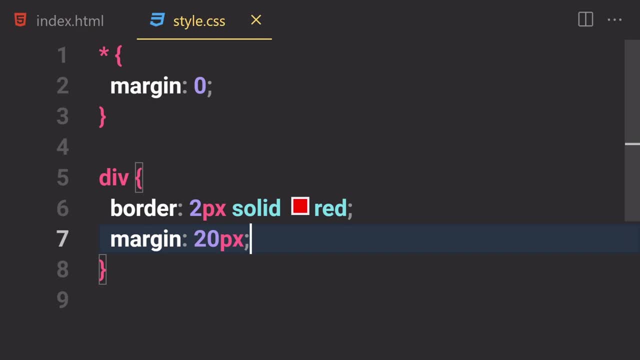 these values by yourself. and now the next topic which we are going to be learning about is something called a css- uh- background properties. so now we already know a lot about css background properties. so now, we already know a lot about css background properties- uh, how to work with the background color. but for now, what i'll do? i'll just select everything and 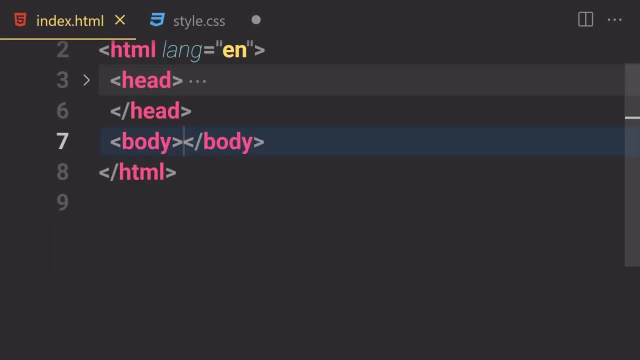 remove there, okay, and i'm going to also remove this box from there. so both of these files, and we don't have nothing inside this body right here. so we have one indexhtml file and css file right here. so now, let's suppose, if you want to work with the images or background properties, to be precise, 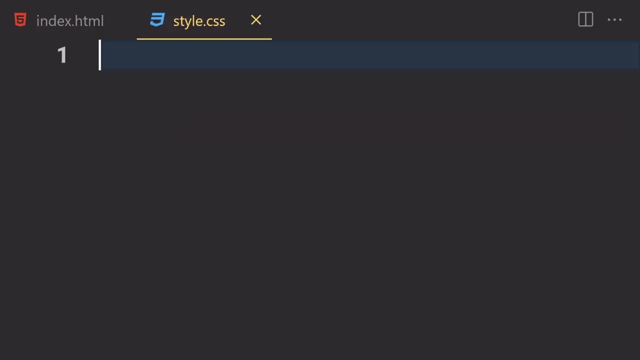 so for that we have to first of all write a div right here. and if you save that- and now let me just select my div inside there- and what do you have to do? we have to just write like higher 500 vh. so if you write a height of 100 vh and if you save that, we will still see nothing because we 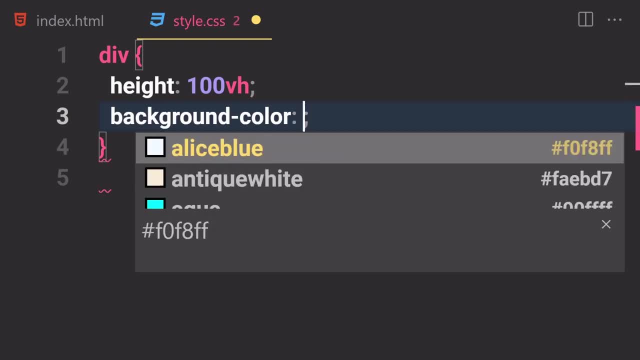 don't have any background color to it. so if you just write a, b, g and c, so here you can see it along, gives us a background color and we can just write like, uh, i don't know different kind of background colors, like red or green, kind of a green one would be fine or greeny yellow would. 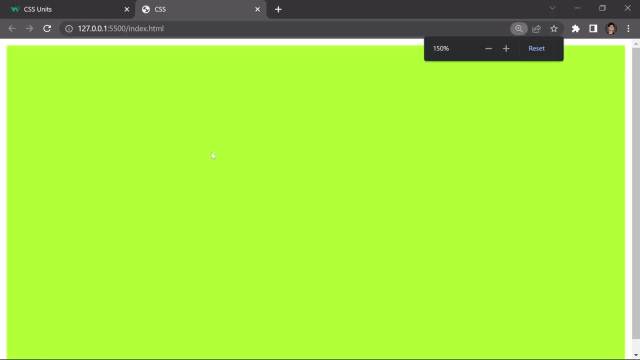 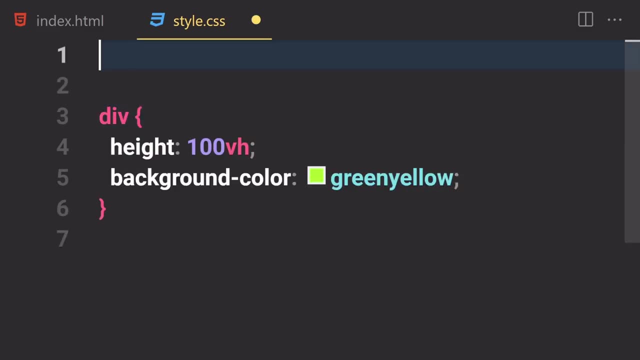 be fine in this case, and if you save that and here you can see, we get this um, green kind of yellow color right here and now. let's just remove these empty spaces from there, like a margin to be precise. so i'm going to select everything and i'm going to just write a. 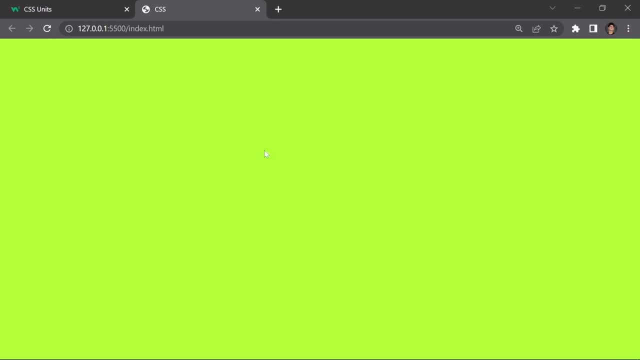 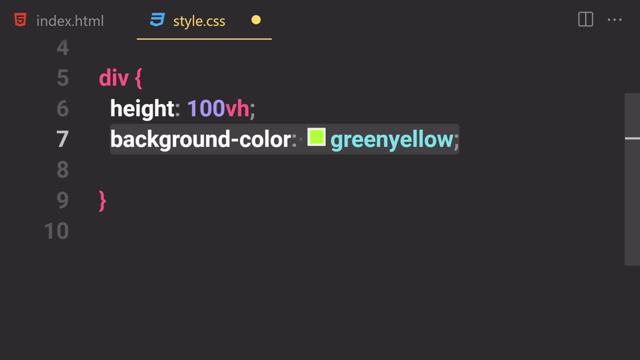 margin of zero to it. so if you save that page, like all of our viewport is now taking this uh, greenish kind of yellow color right here. so now we already know, like, what is this background color property will do for us? background color property will just change the background of our container, or 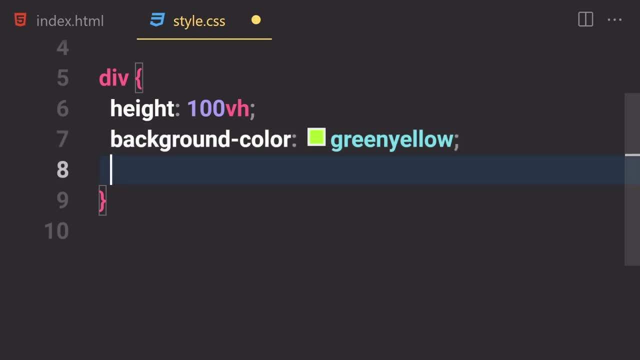 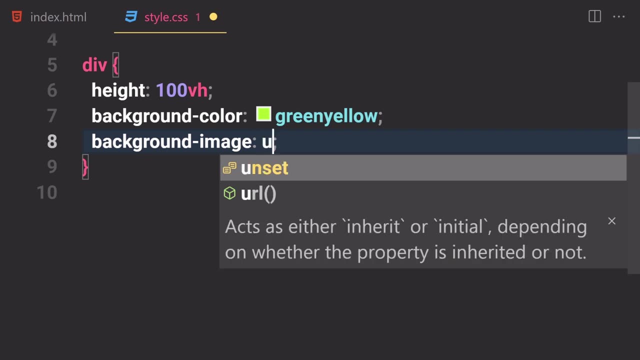 box, whatever you want to call it. okay, so now, the next property which i want to talk to you about is something called a background image property. so if you just write a background image and here we have to pass a url, a uniform resource locator, you don't have to worry about uniform resource. 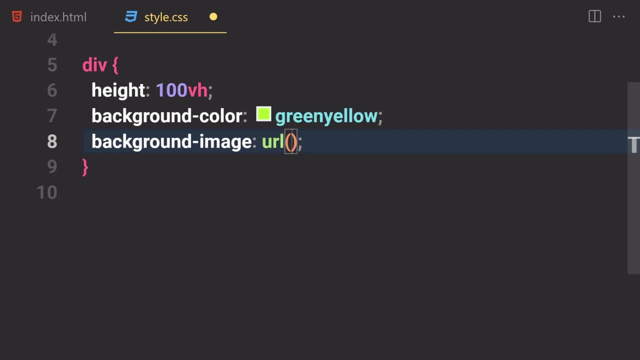 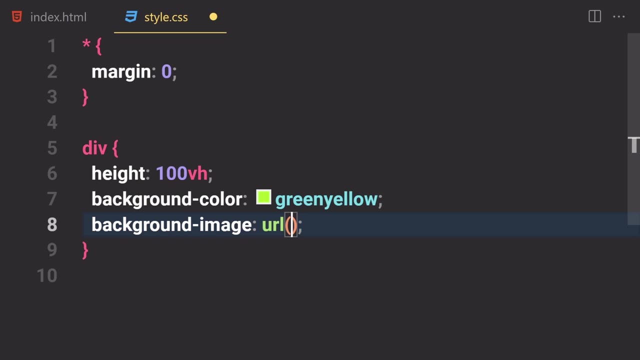 locator, but here it will ask us about a location of the image. like, this property allows us to provide image to that specific kind of like div or the header or anything you have selected. but now, in this case, we want to provide a background of image to this div, so for that we can use this. 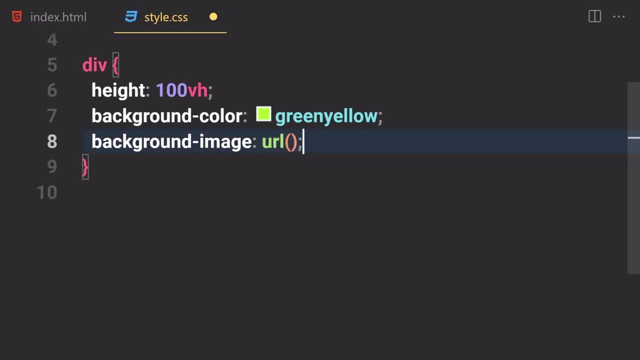 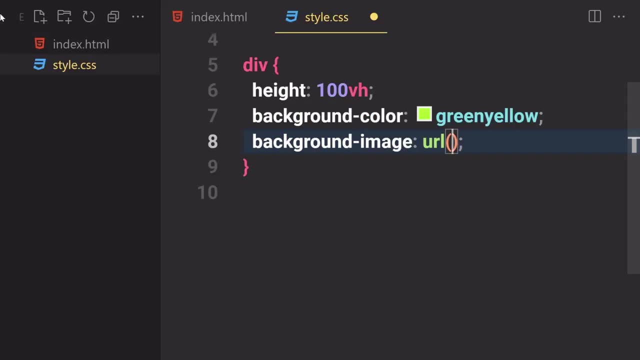 background image property and then this url. and here we have to specify the url of that image so you can use remote url or local url, as we learned that in a previous video, like, if you have your own image, so you can provide that path by holding ctrl and heading space, so we don't have 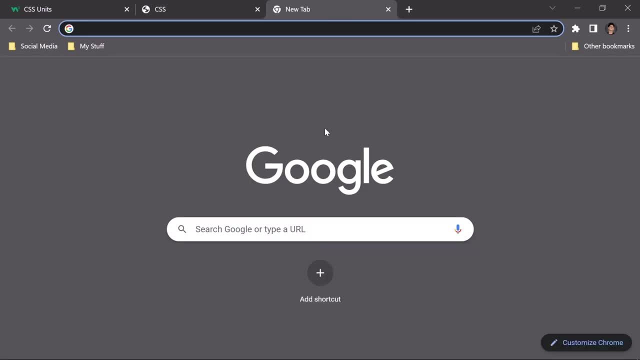 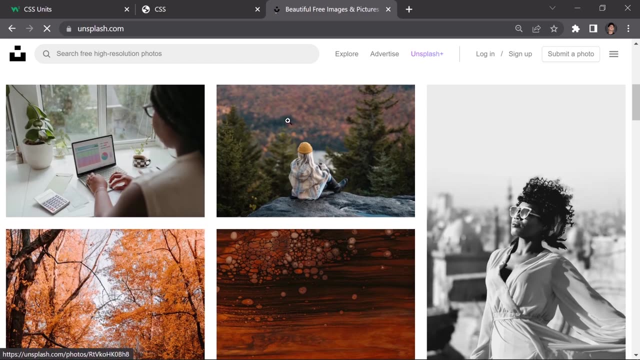 any images for now. so we are going to be using a remote uh path. so i'm going to just write like unsplash right here and i'm going to go to this unsplash and here, let's suppose if i want to get this image, so i'm going to click on that and shout out to this person: sorry, i can't pronounce your. 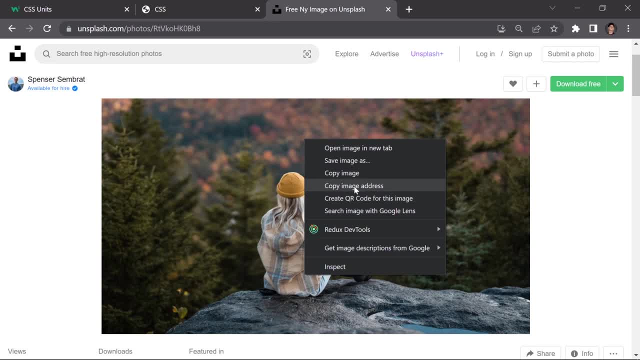 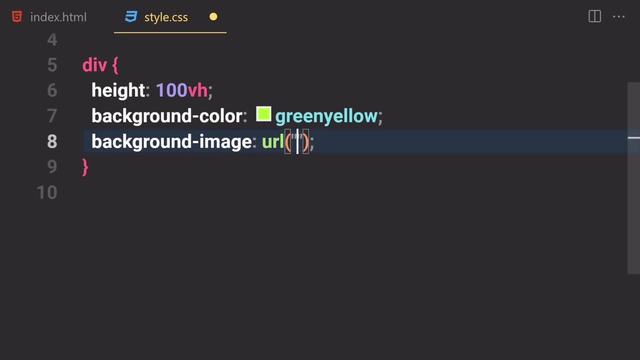 name, but i'm going to take your image and thank you so much for this image. i'm going to copy this image address from here and what i'll have to do i'm going to have to provide a quotes in there. so if i just write a quotes and then here i'm going to have to paste this link. so i'm going. 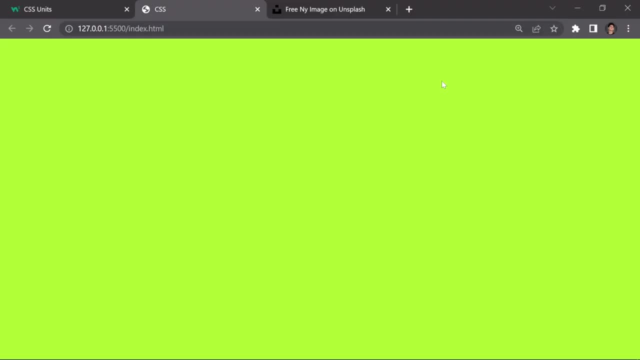 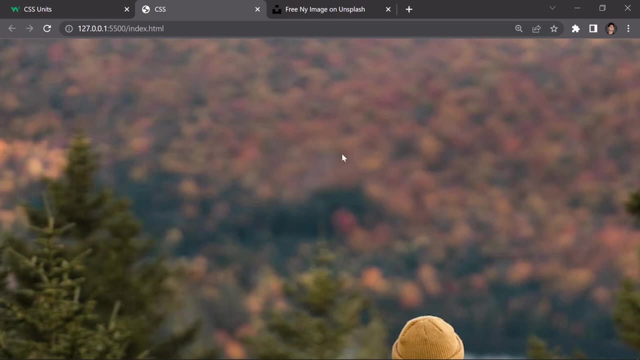 to zoom out of it and this is how it looks like, and knife is server file and boom, we have this image right here. but there are different kind of problems in these images. which kind of problems do we have? well, um, the first thing is that it's not repeating itself. so, first of all, 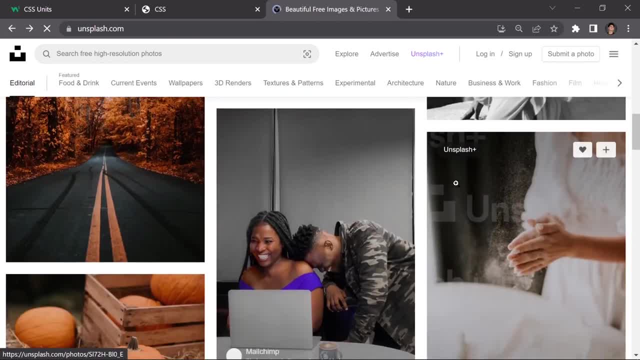 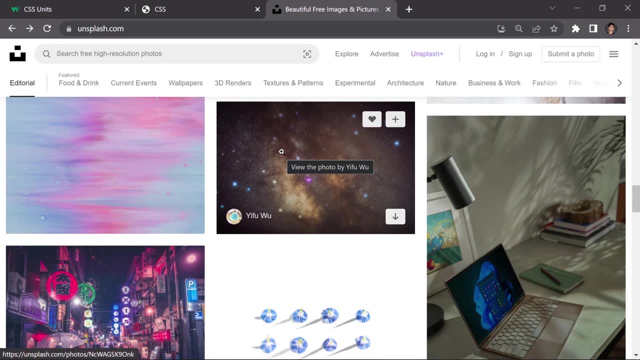 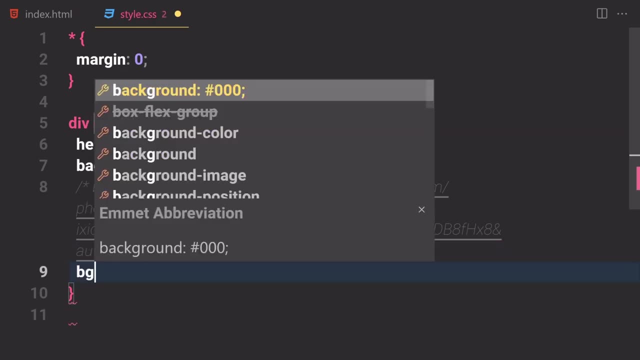 let's just find an image which is repeating itself. so i don't know which kind of image would be fine which is repeating itself. maybe this galaxy would be fine if you copy that. i really like this image. so i'm going to comment this line out and i'm going to write like a background image and then url and here: 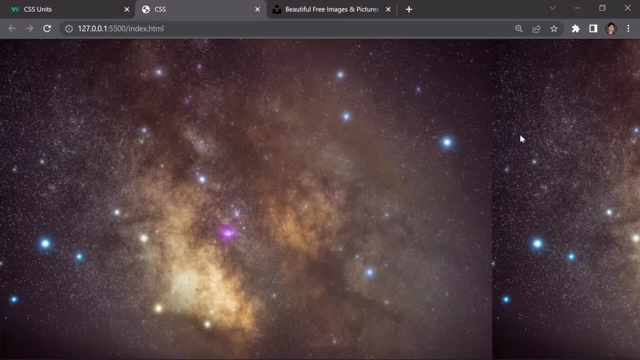 i'm going to pass this link right here, so if you sell that, all right. so now, here you can see, this image is now repeating itself. so we have this image like a sky, and now, here you can see, this is n right here, but we also can see this image right here again, so this is now repeating itself. 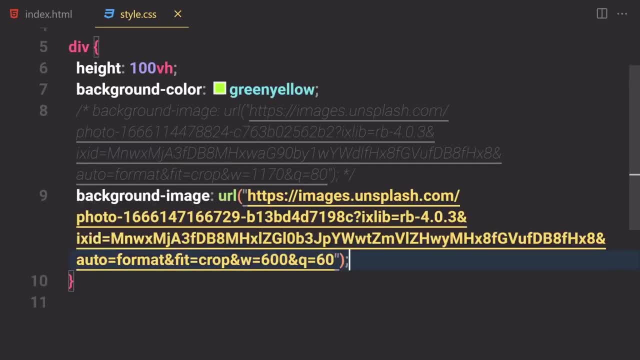 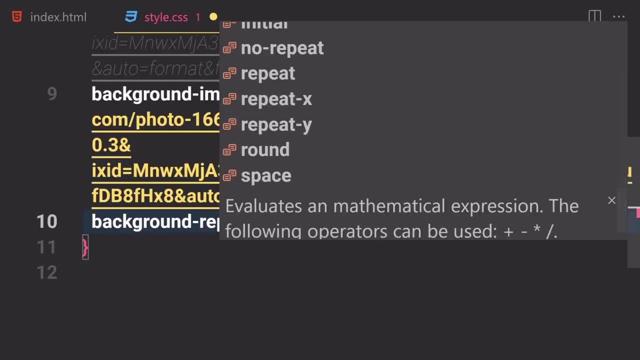 so if you want this image to do not repeat itself, so for that we can use a property called a background repeat property, and here we have different kind of uh repetition properties, like we can repeat for the x-axis, if you want to like, repeat x and if you save that. 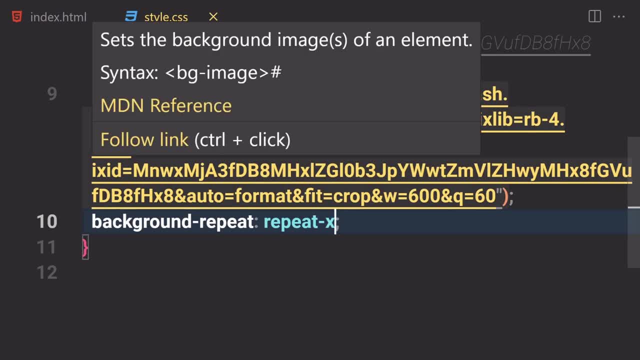 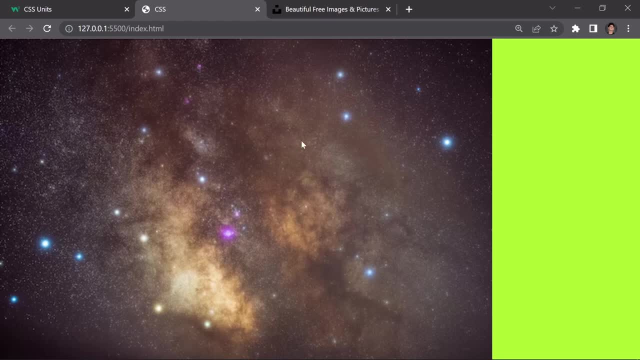 and it will now just repeat for the x-axis. right here we can repeat for the y-axis, so if we save that, so it'll now just repeat itself for the y-axis. but the image is a little bit bigger, so that's why we cannot see that right here and we can also just provide a repeat of non-repeating. 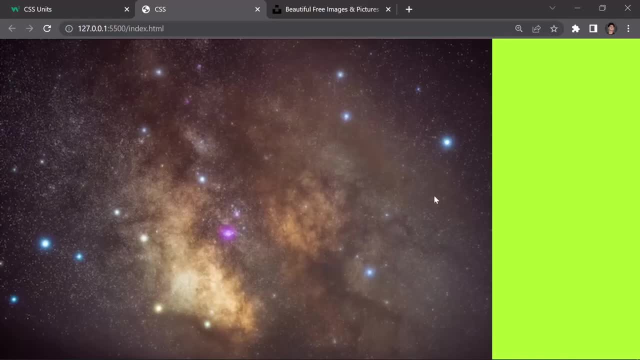 our no repeat, to be precise, so we can just write no repeat and it will not repeat itself. and now, here you can see another problem. which kind of problem we have here you can see, this image is now at this area, but we want this image to take its entire space. so how can we go about? 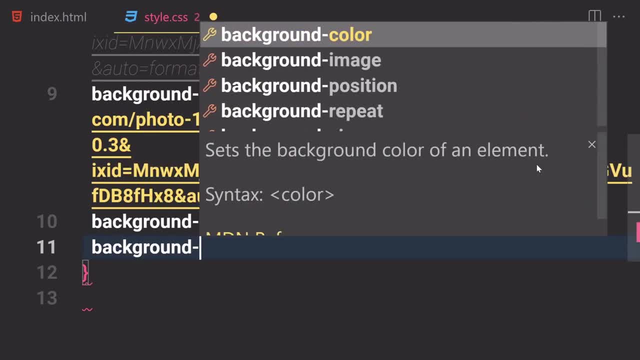 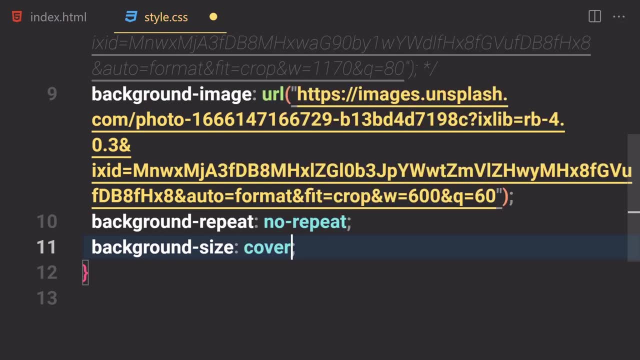 doing that. well, we have another property of a background. so if you just write background of size and here we can see we have like auto contain cover and stuff. so if you just click on the cover one and if you save our file so here you can see, it will now cover this area. 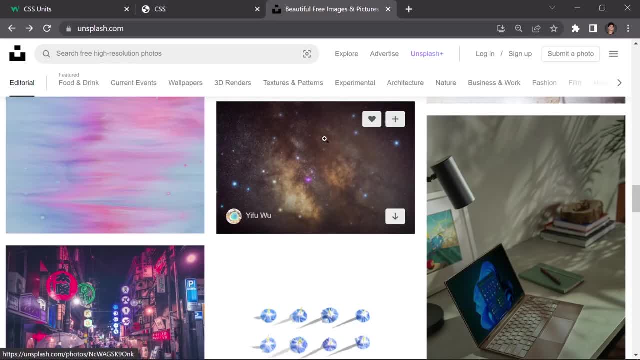 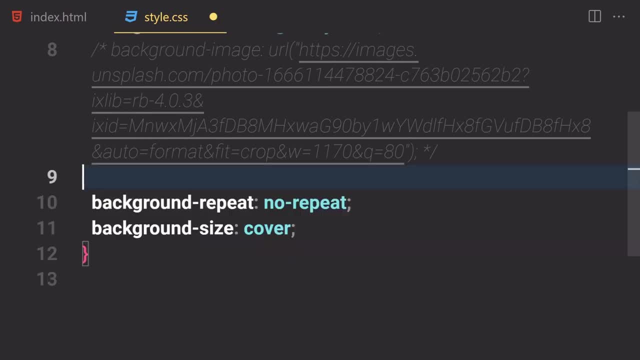 but we cannot see that upper bar right here. it's kind of awful image. you know, i'm going to remove this image real quickly, because we already learned about a background property. i mean like background repeat property. i'm going to remove this one, i'm going to uncomment this picture, save our file and 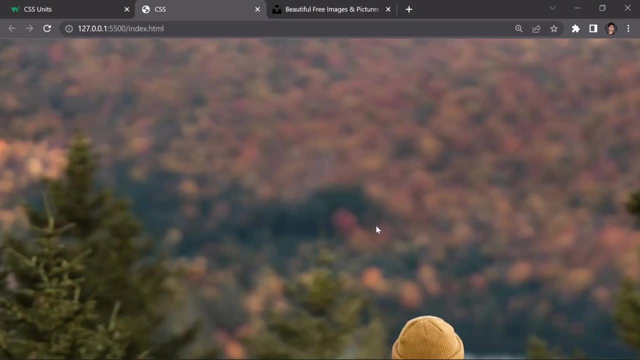 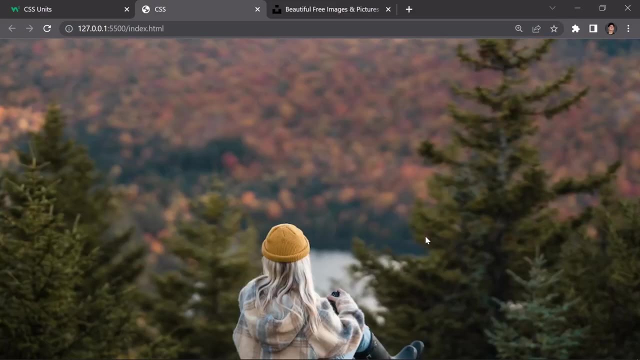 now here you can see. if you just comment this line of code, save our file and this is how it looks like. and now, if you want to cover the background size, so we can just use like background size cover, and if you save that and this is how it looks like, now we have another problem. now we can see her image right here, but 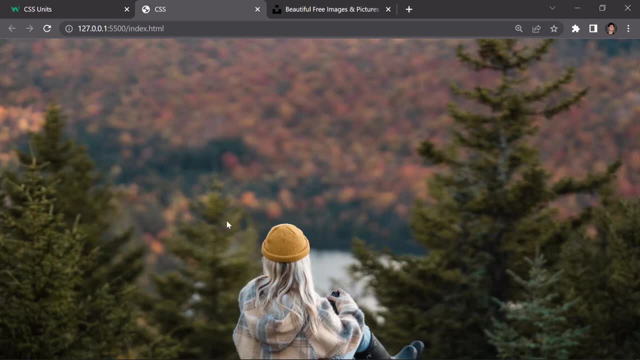 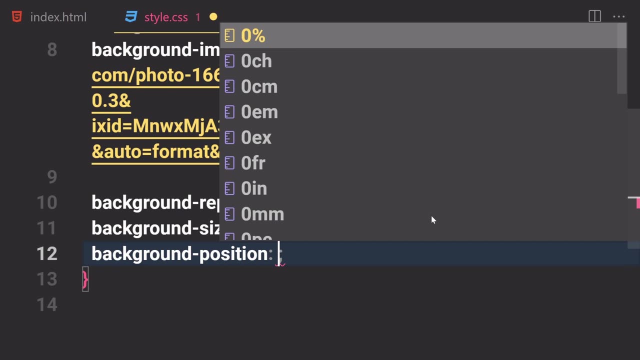 we don't want this blurry kind of area right here. we want her image to be inside this area. so for that we can just use like a background and then position, and here we can specify to the top, to the bottom, to the left, to the right. so let's suppose, if i just want right for the bottom, 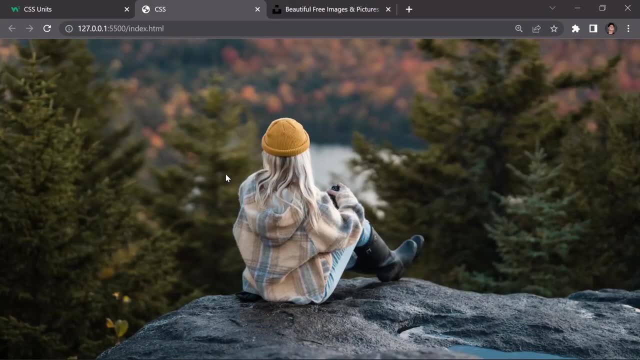 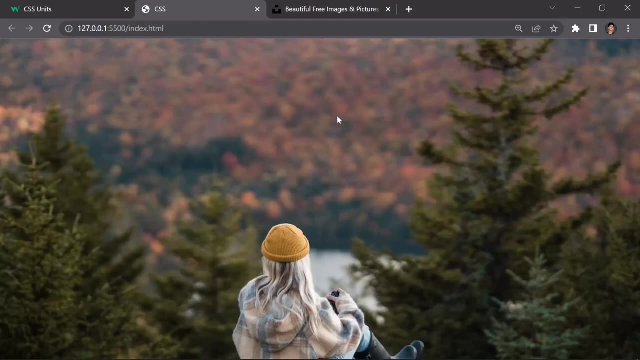 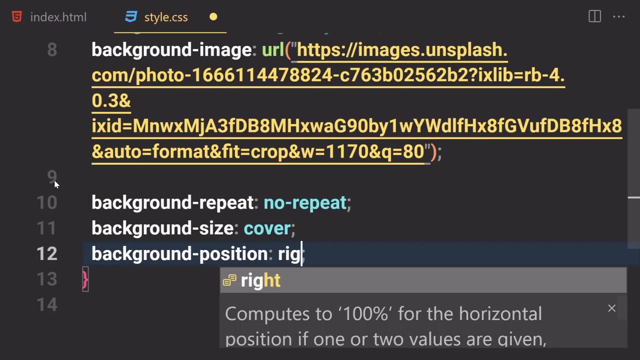 and if you save that and boom, now we can see her image and we cannot see that blurred image like above the sky image. so we can just write like top to get there and this is how it looks like. and now, if you just write like left, so if you save that and this is how we get our left area, we can also get for the. 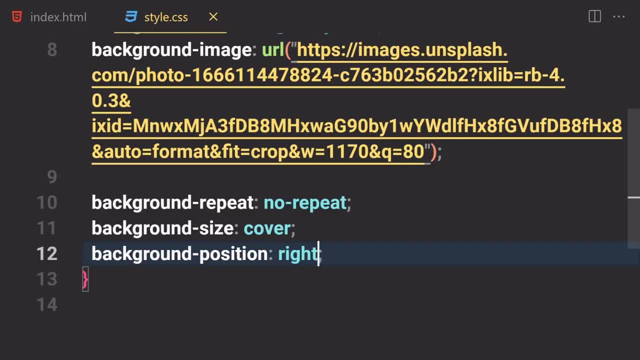 right area by just specifying the right area, and now we can see the right area. we can also put a center, if you want to save it, and it will now give us the center of this image. but uh, in my guess i'm going to just stick to the bottom one cell file. and this is looking cool for now, right? 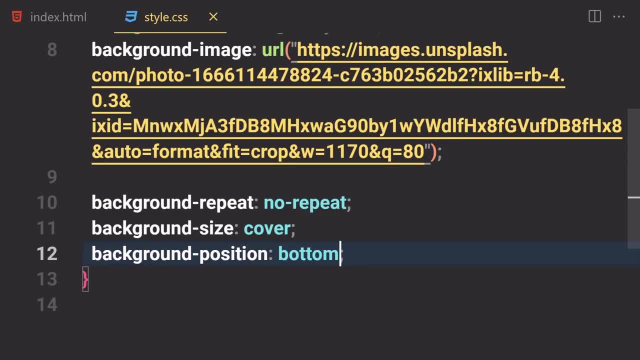 here, okay, so so now that we saw a little bit of problems using this image, we can just save it and we can just use the background image property and we can just use the background image property. so background image property allows us to, uh, specify the image or provide an image to our 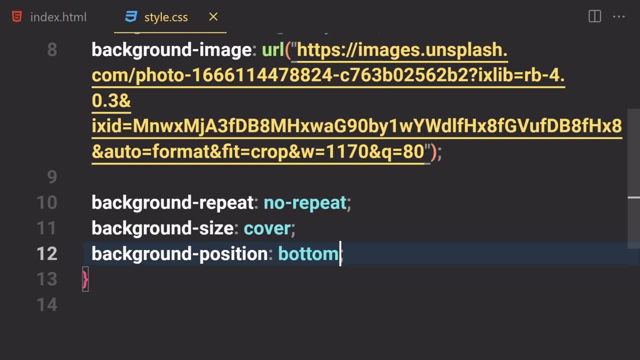 box. then we have a background repeat and if our image is repeating itself, so we can also remove the repetition of their image. if our image is not totally covered, so we can use a background size covered, so we can cover that and we can also use background position property. but now the next. 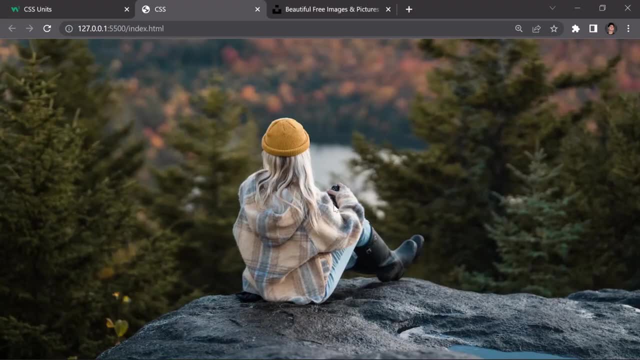 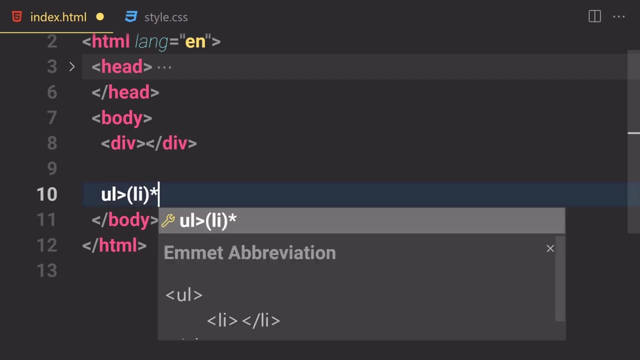 thing i want to do is that i want a parallax effect on this image. so now, in some cases, if i have like a lot of, if i just write uli, and then we want like uh, 50 li's and if you sell a file, so here you can see. 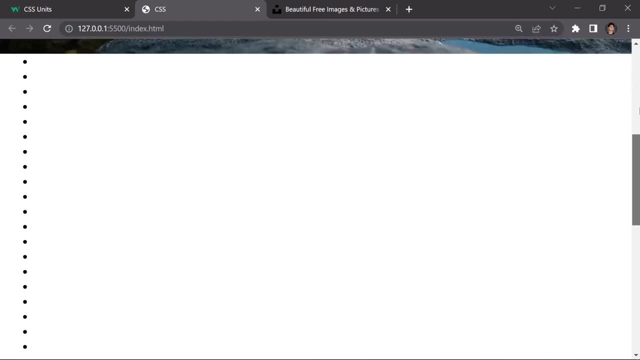 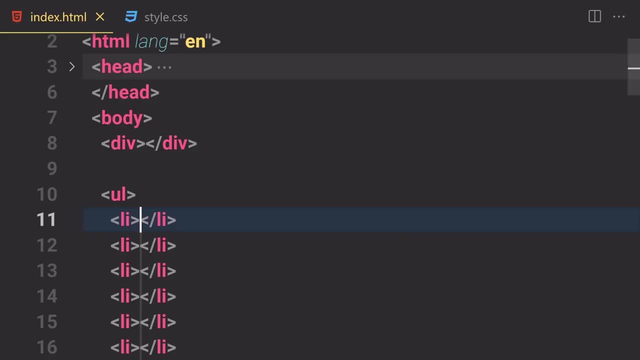 the log uses like 50 li's right here. so we have now this scroll bar right here, so anytime i scroll, so this image is not scrolling with me. so if i want that kind of effect, so for that we have another background property which is called background attachment. so if you just write like a background, 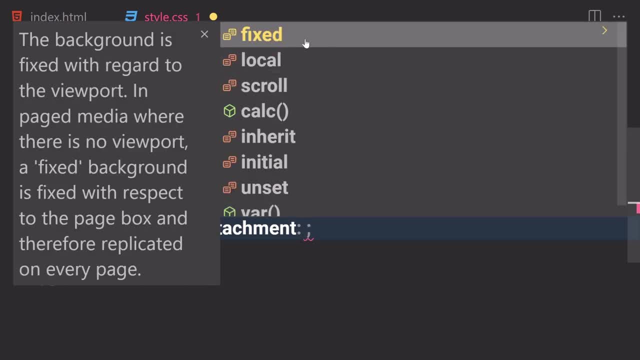 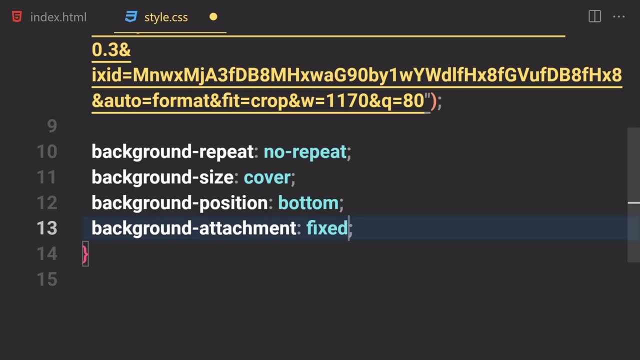 attachment property and we have a few values for it. like we have fixed, we have local scroll and you don't have to worry about any other of them. but in my case i'm going to just click on this fixed one and if we save a file, and then now if i just scroll down, so here you can see, that image will stay up there and we will get. 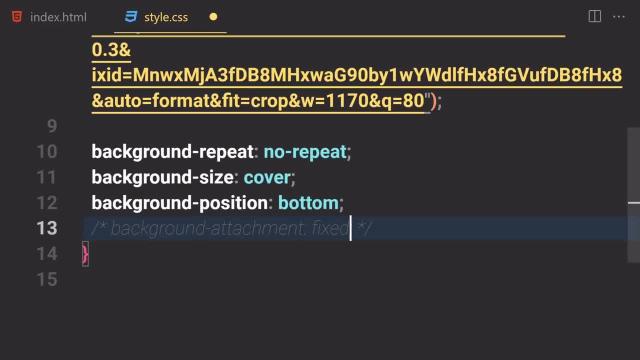 kind of a parallax effect right here, if i just comment this line out and save a file and if i scroll, so here you can see this image is scrolling with me. but if we don't want that, we don't want that kind of a parallax effect if we save that. and now if i just scroll down and here you can see, 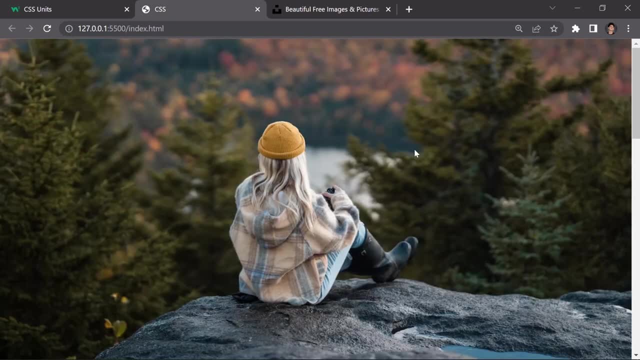 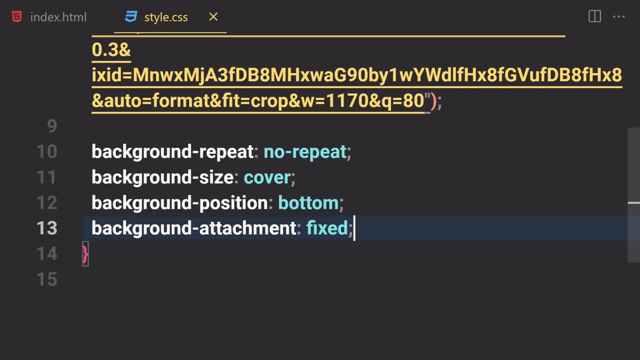 that image is also scrolling with me. not i mean like this image is not scrolling with me, but it's giving us this kind of a parallax effect right here and now. let me just show you the final thing about the background property and which i will not recommend. 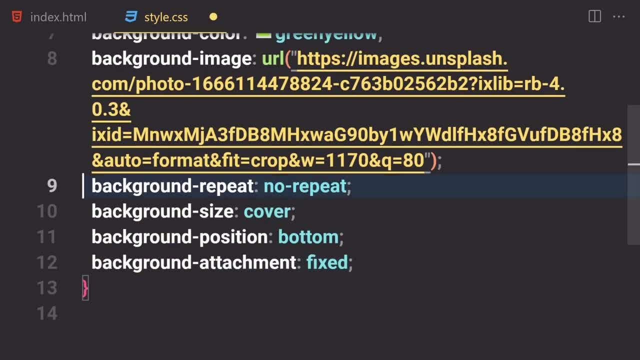 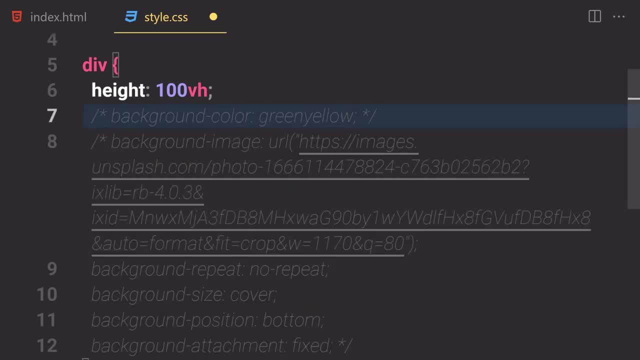 you to use that in your projects because it's confusing a lot of the other developers and also yourself including. so i'm going to just remove or not remove. i'm going to comment all of this area. i'm going to also comment that background one. save it so we can use a background. shorthand property. 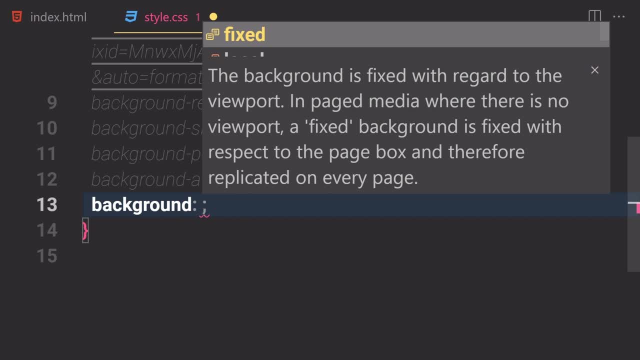 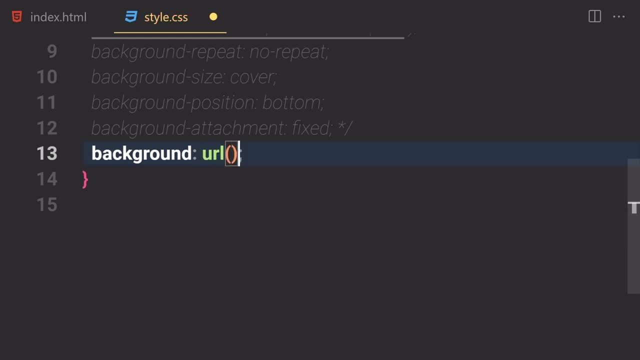 but, as i said that, i will never recommend you to use this property in your own personal project or someone else project, because it confuses a lot of developer. so the first value we have to provide is a url of that image. so in my case, i'm going to get my new kind of image. 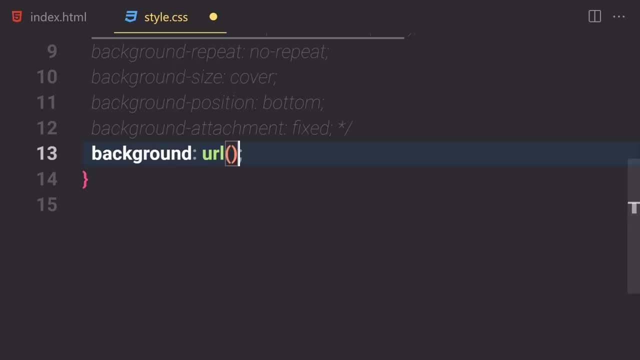 like, uh, i don't know, i'm going to right click on it and copy this image address. or, you know, i'm going to click on that so we can get a high quality result and then copy image address and then here in a quotes i'm going to just provide this image in here. 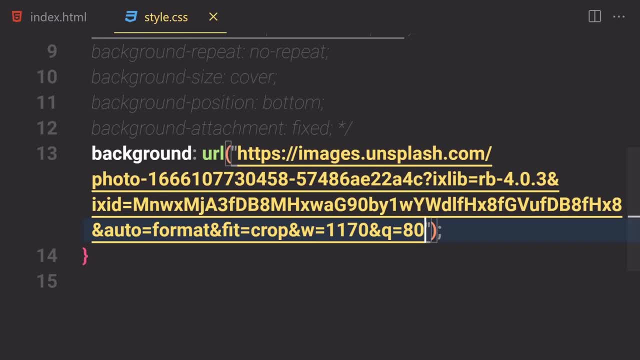 so knife is cell file and here you can see we get this image right here. but now here, the another property which you have to provide is something called no repeat, which we just learned, and this is a position uh, background repeat property. so we have to provide this value. 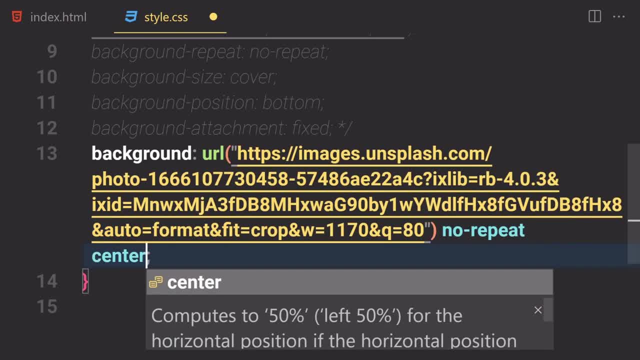 then now the next property we have, or the next value we have to provide, is a center, and center will be for uh, background position property. in this case we provide bottom, but here we are now just providing a center. you can also put um bottom if you want to. now, here we just have to write a. 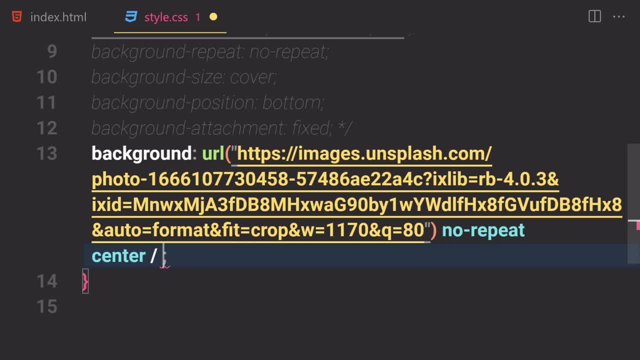 slash, and then we have to provide the value of this background size property. so what do we have? we have a cover, okay, so then, finally, we have a background attachment property. it's value. so i'm going to just write a fixed in here and knife is out there. 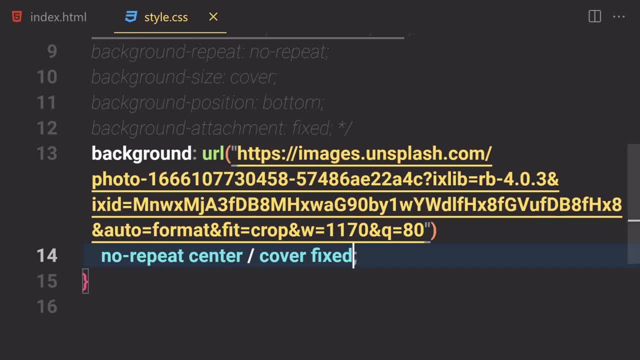 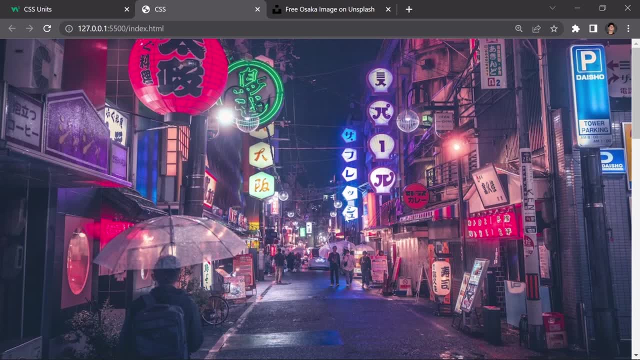 and this is how the image looks like right now. okay, if you want to get the bottom results, so we can just remove that center and we can just write a bottom, and if you save that, so here you can see, it will not use this bottom area right here. okay, and you can play around with this image. 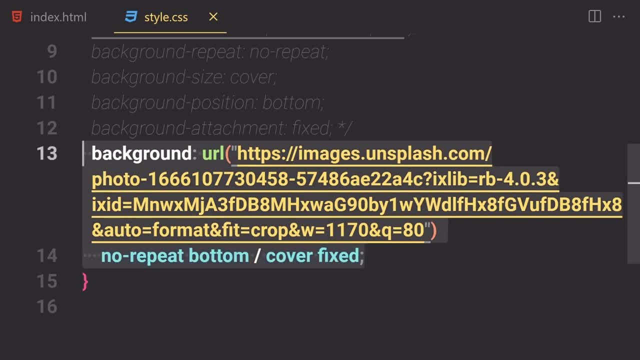 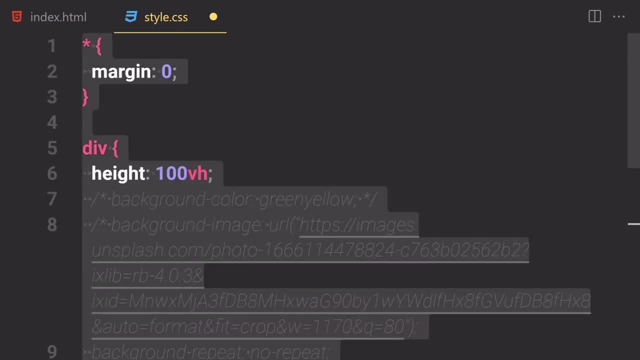 as you would like, but i will never recommend you to use this uh shorthand property, but i just kind of want to show you like this property do exist. i'm going to remove everything from this div, or you know everything except that uh resets. i'm going to remove everything from here. 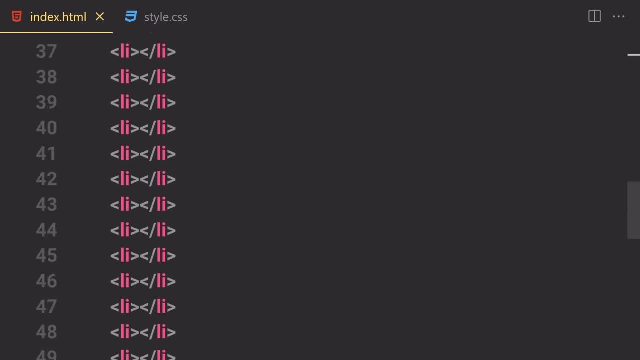 and now we are totally done with the background property in css. so the next topic which you're going to be learning about in this video is something called, uh, gradient and filters. so if you want to provide a gradient, so first of all let me tell you like what in the world is. 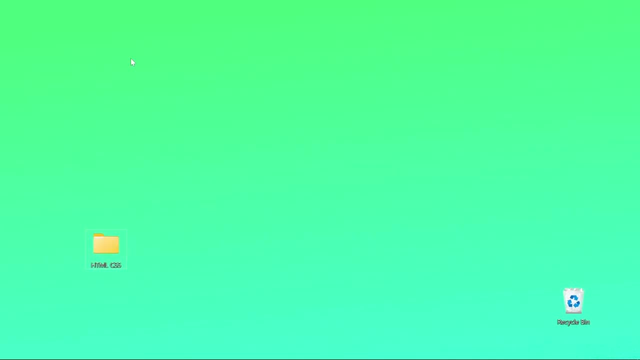 a gradient. a gradient is like this color. let me just show you that here you can see we have the mixture of colors, like we have a dark green right here and we have a gradient here and we have a little bit slighted green right here. when we mix two colors at once and we use that in some sort of 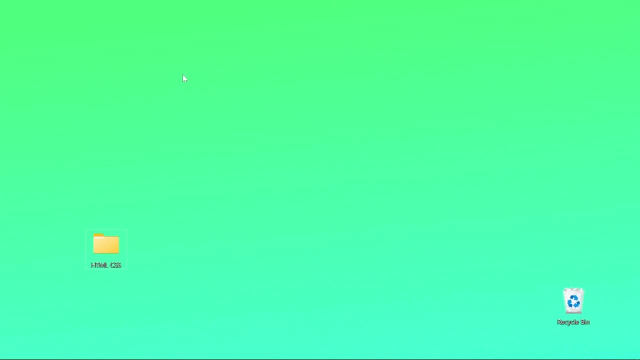 element, so that is known as a gradient. so like not just two, two colors to be precise. if you use like more than one color at once and we just specify that or use that in some sort of element, so that is known as a gradient. so these are now two colors, but we can go like three colors, four colors, and so 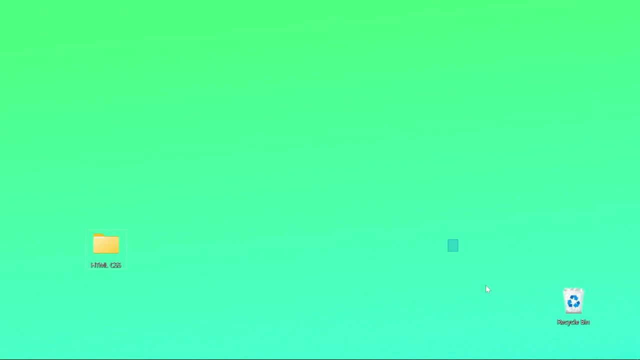 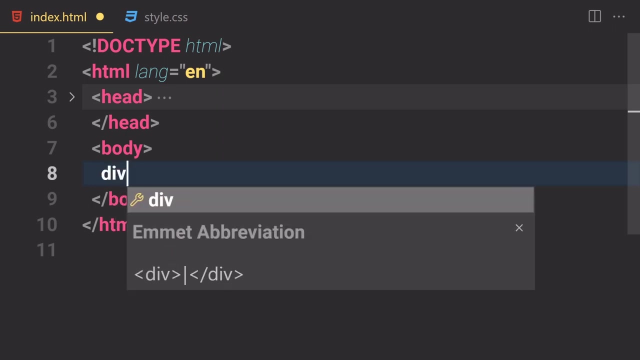 on and so forth. so this is now totally a green color and this is a little bit grayish kind of green color, and so now let me just show you all of that in action, then you will get to know what i'm talking about. so if you just write like a div in here and now, if you want to provide a gradient on some sort of 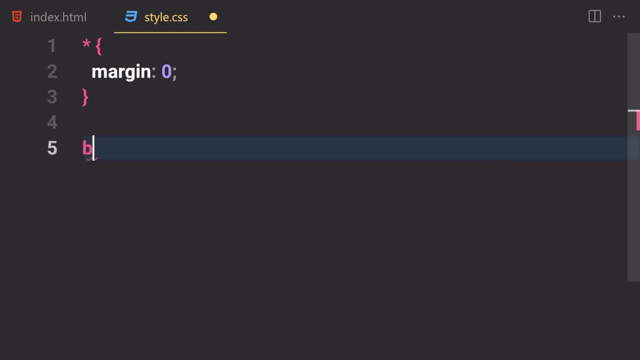 image. so first of all, let me just get, uh, some sort of image. so i'm going to select this div and now, here we are going to be providing a background of image right here and now. let me just put an image like url. let me just get some sort of an image. this one isn't cool, so 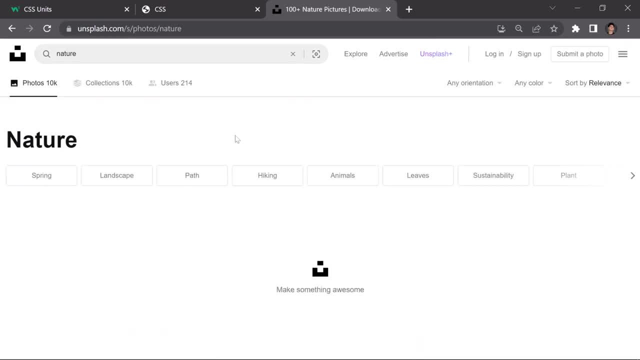 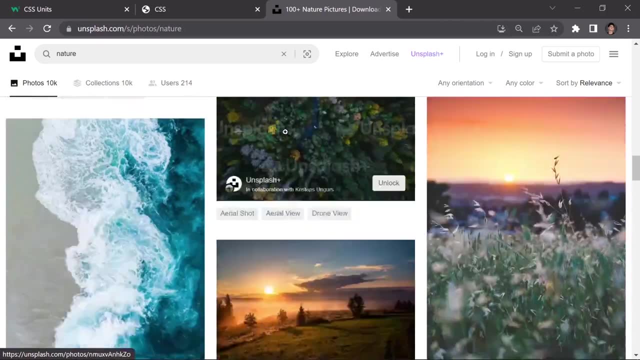 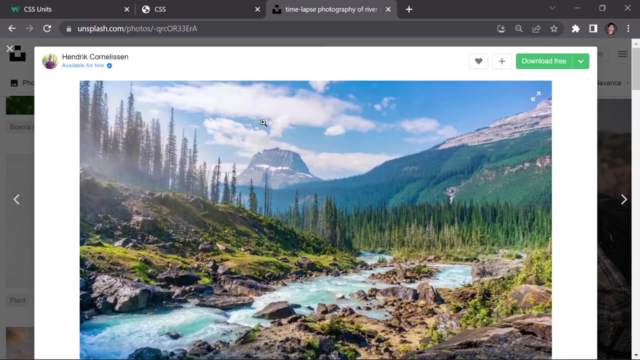 i'm going to search for a nature real quick, so i'm going to click on that and go to a nature, and which kind of image would be fine. now let me just see, you don't want, i really like this image. so what i'll do? i'll just click on there and then i'll right click on it and copy the image address. 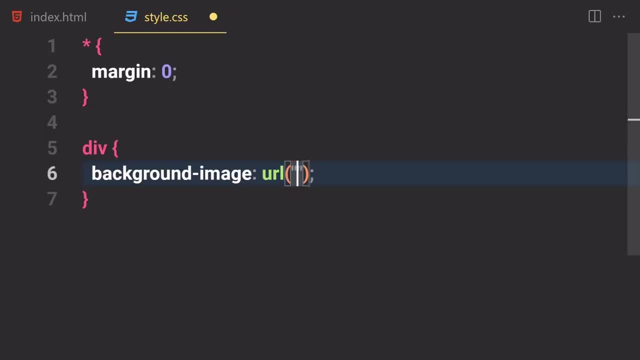 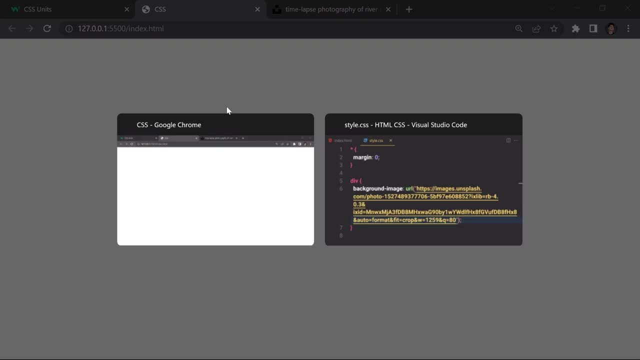 and shout out to this person: okay. so now i copy the image address. i'm going to just write my quotes and paste it right here. so now, if you want to provide a gradient on this image, oh my god, first of all it have to be rendered. okay. we didn't provide any height stir, so i'm going to just 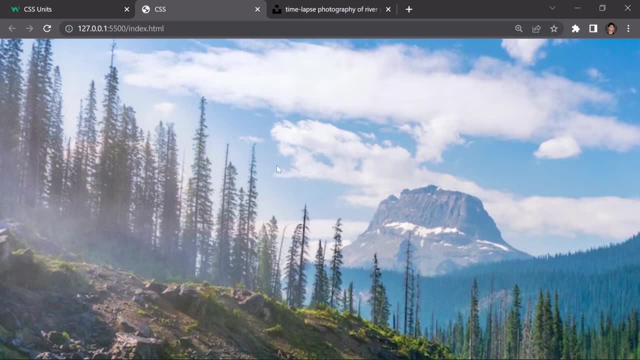 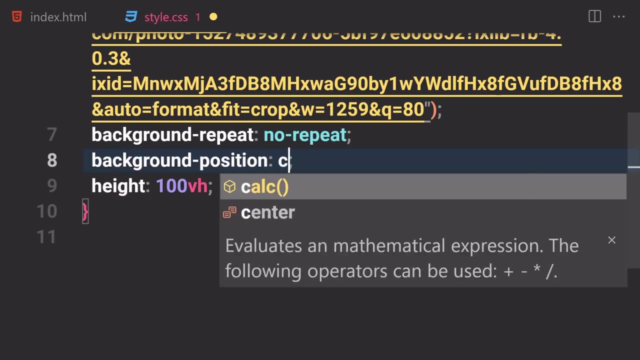 write height. so height of 100 v, yet seven, oh my god. first of all it have to be rendered okay. we yet save it and now we have our image. so now let's just provide our property background repeat of no repeat. and background position will be center. background size will be cover. 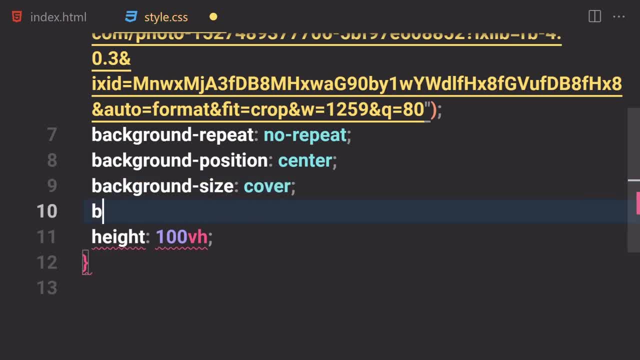 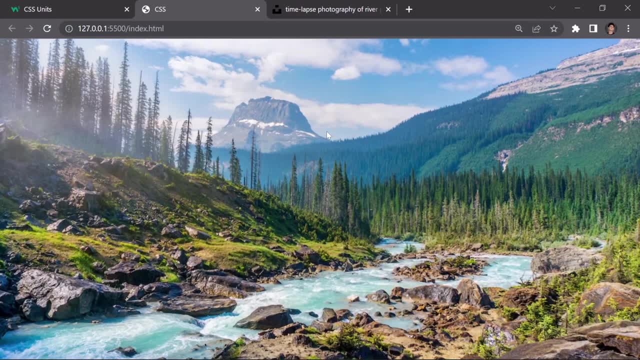 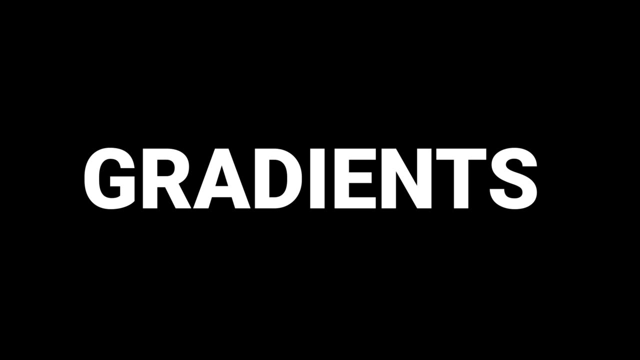 not contain but cover and background. attachment will be totally fixed. uh, fixed server file and boom. this is how it looks like for now everything is looking the way we expect them to look. so now, if you want to provide a gradient on this image, so for that we have to specify. 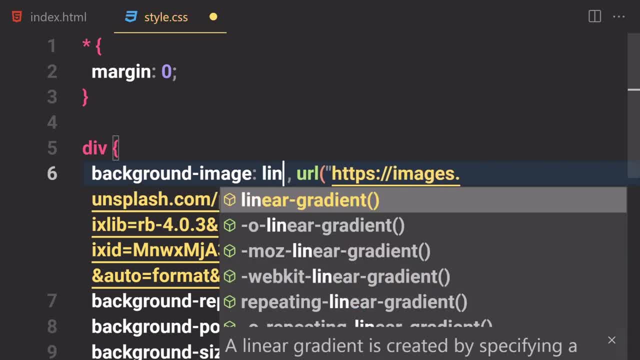 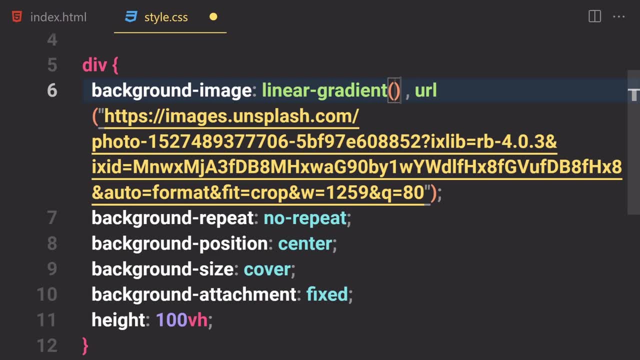 first of all a comma and then here we are going to be writing a linear and gradient. so we have two kind of gradient inside of css. so we have a linear gradient and we have a radial gradient, which we are going to be also exploring just in a second. but first of all, 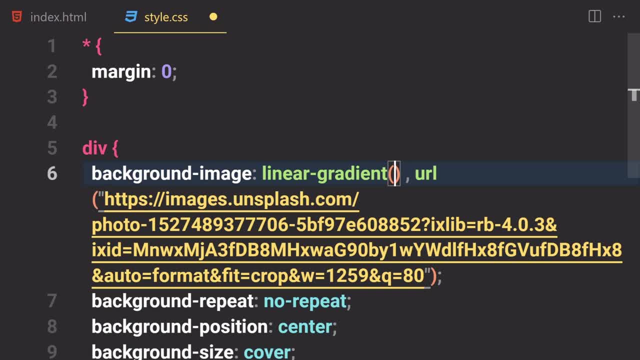 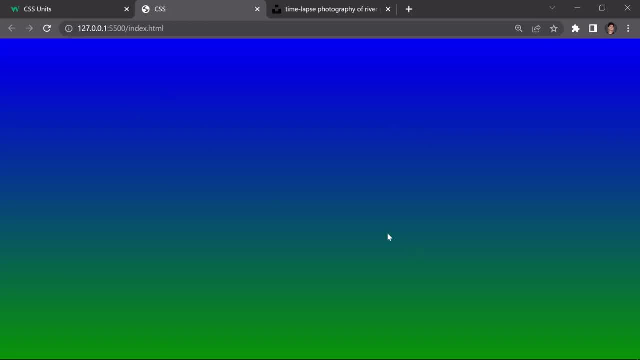 if you want to like work with the gradient. so we have to provide two colored. so let me just write like blue and green. and now, if you save that, and what do we get? we get blue and green colors. so now we get like blue and green colors so we can modify them by using the opacity. so i'm going to 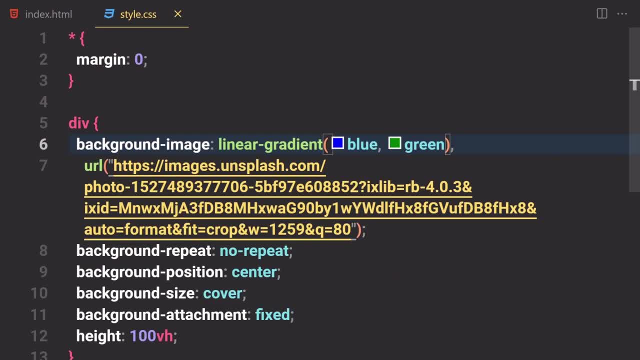 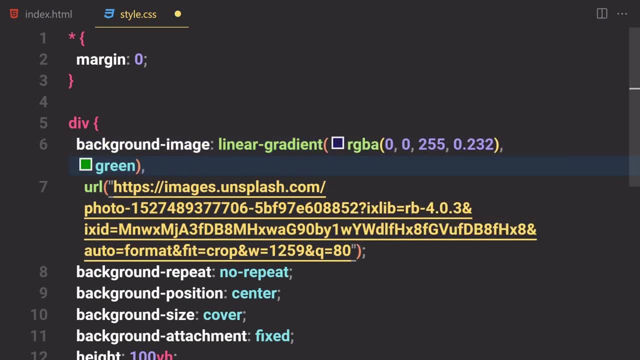 just, uh, zoom out a bit so you guys can see everything a bit better. i'm going to hover my mouse over to this blue and i'm going to change the opacity to be like so, like that much. so here you can see that opacity and i'm going to also decrease the opacity of this one. and now, if you, 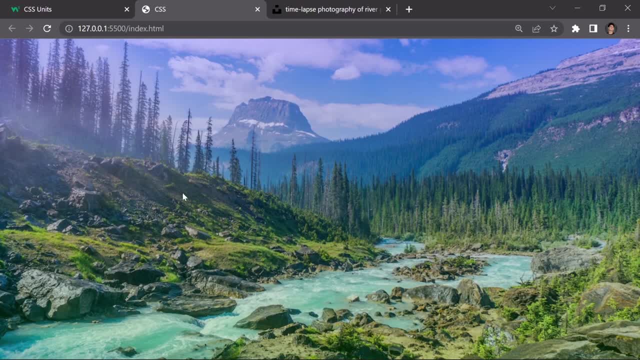 save that and here you can see. now we add our gradient right here inside this image. okay, so if i just like, let me just cut this uh gradient from there. let me also cut this comma from there. if you save that, and this is how it looks like image by default, but if you want to provide a 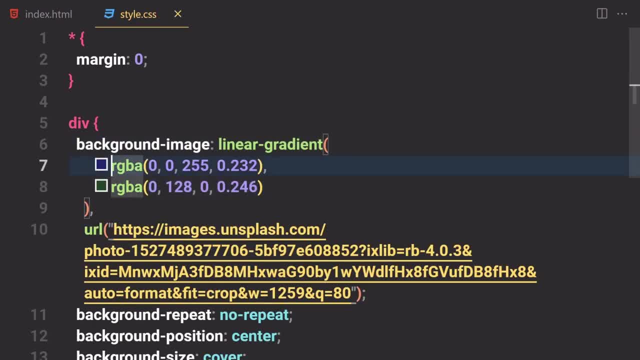 gradient. so this is how we can provide a gradient: you can choose whichever kind of color you like. let me just write like maybe red kind of color and if you just lower its opacity to like so, and we have green color. so i'm going to select a kind of a bluish color. 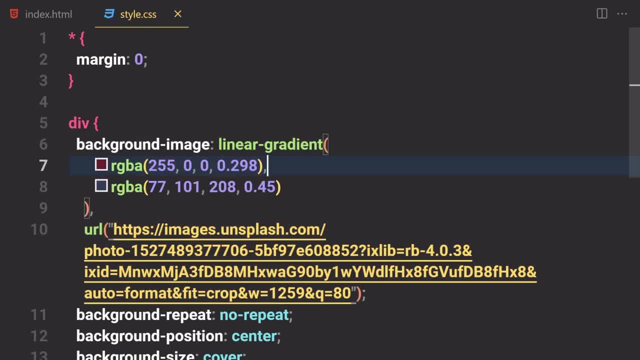 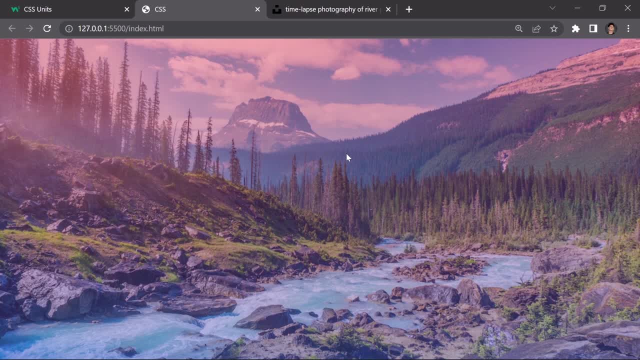 and lower the opacity of this one, maybe like that much. and now, if you save that and boom, this is how our image looks like right now. okay, so you can play around with. the gradient is a linear gradient, so which means that we can change its uh positions as well, if you want to. 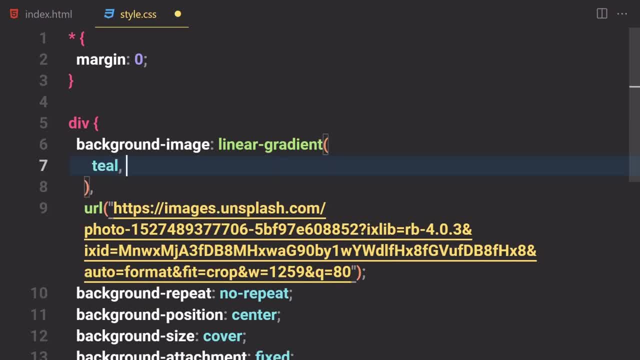 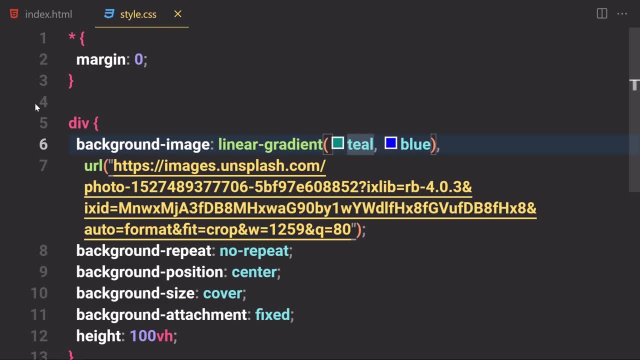 so you know i'm going to remove that and i'm going to just write like: uh, teal and blue, and if you save that and here you can see, we get a teal and blue color right here. so if you want them to be like from the left, so we can also write to left and then comma. so if you just write that, then we. 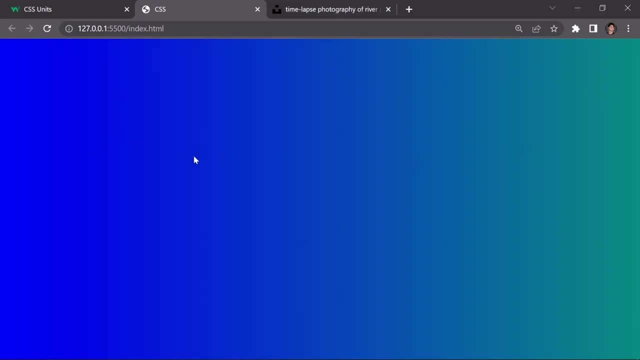 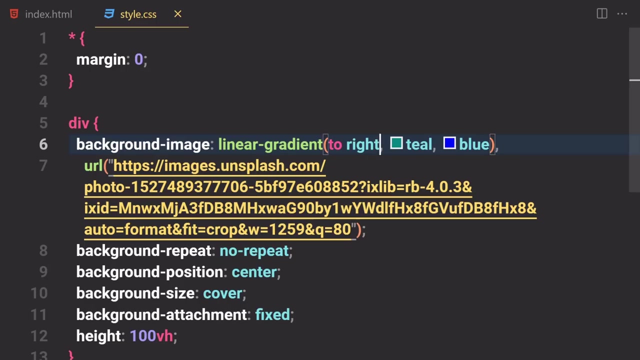 have to save our file. and now here you can see the log uses this color from the left, right here. if you want this color to be from the right, so you can just write to the right, and if you save that, it will not gives us this color to the right. if you want them to be for a top, so we can. 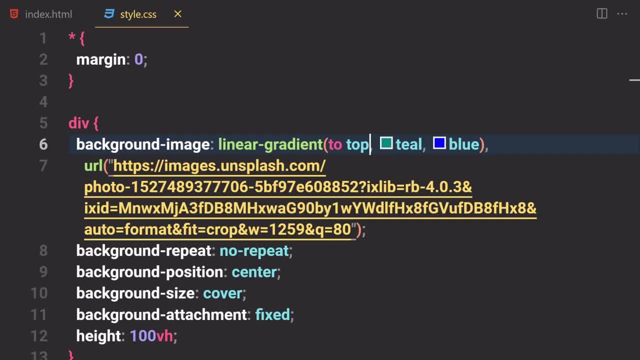 just write to the top and save our file. it will not use us to the top if you want them from bottom, so we can also just write a bottom. it will not give us this color as a bottom. okay, and we can also specify more than two colors, like uh, i don't know, red would be fine. and now, if you save that, 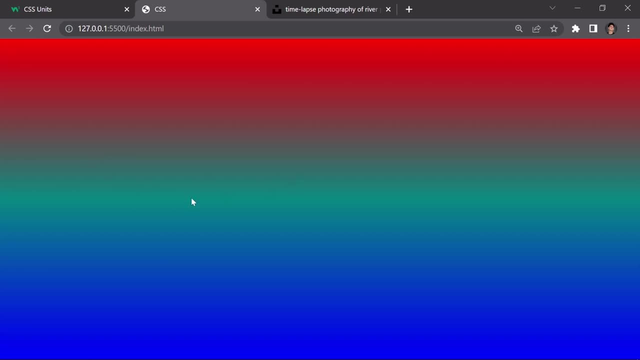 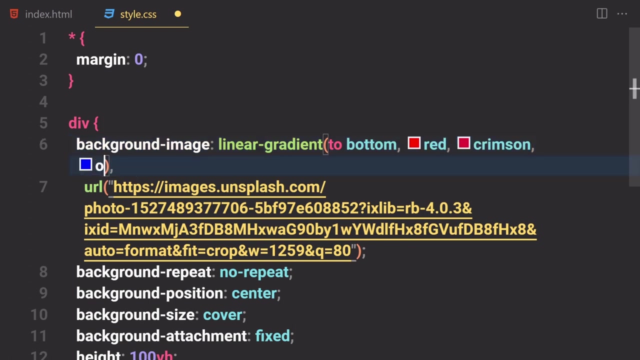 so here you can see, now we have three colors. we have a red teal and this blue color. so maybe i'm going to change this one to crimson kind of color and this one to be like orange. so if you sell that and here you can see, we are now getting this kind of uh effect. so we 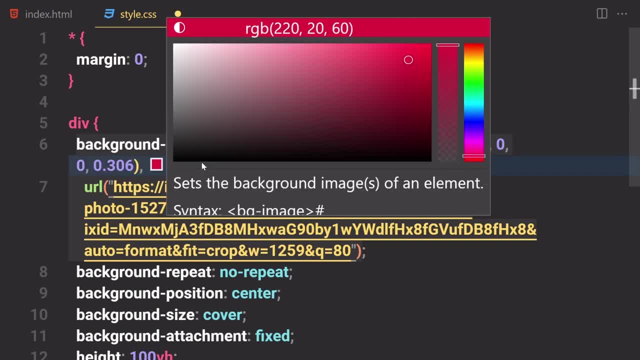 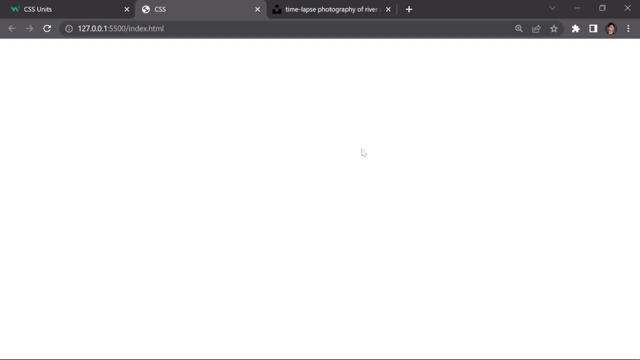 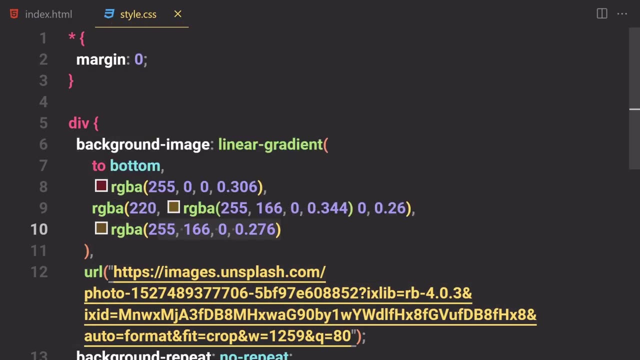 can lower the capacities if you want to. so we have a crimson. we have this one kind of orange, so maybe like so, so i'm going to sell that, okay, so we messed up something inside this orange. one lower the opacity is severed. we did mess it up something. you know i'm gonna. 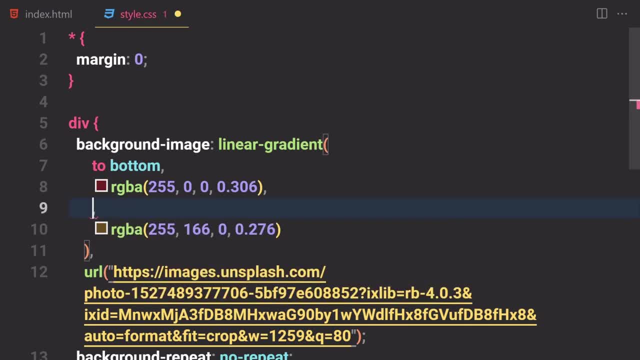 remove this crimson kind of property. let me just write crimson, scrimson property and this is how it looks like. now let's just change the opacity of this one to be like so severed, and here you can see we are now getting different kind of results. so this is how. 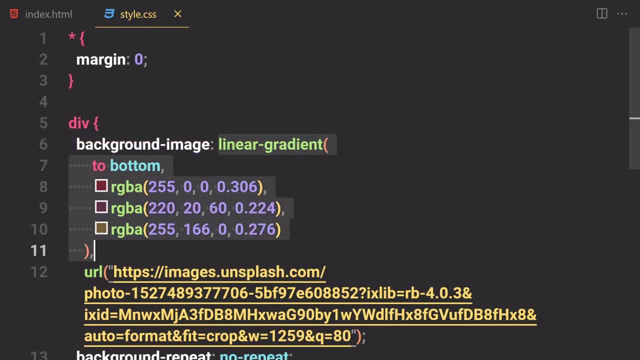 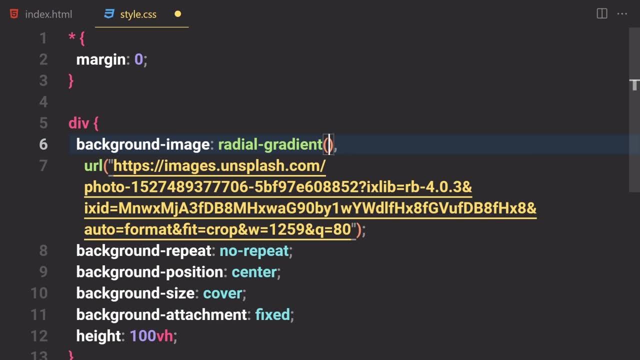 you can work with a linear gradient. now let me just show you a radial gradient. so i'm going to remove that and instead of linear gradient we have to just write like a radial gradient. so here we can just also provide a different kind of color. so i'm going to write like blue and then sky blue, and 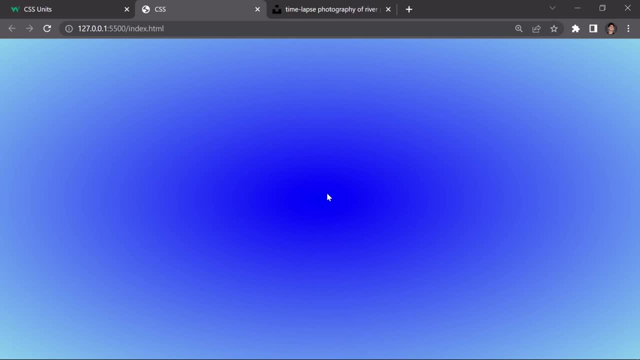 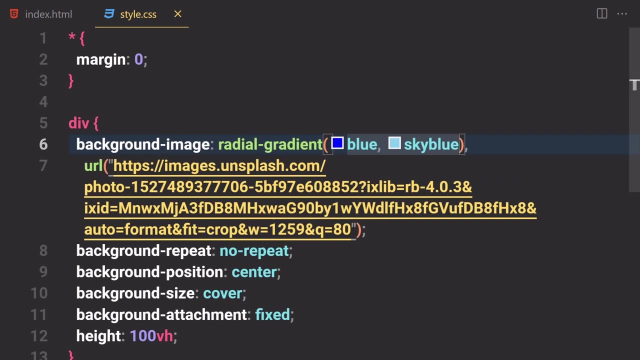 if you save that, it will also give us like a sky blue, but here you can see, this blue is kind of a circle coming from the center right here. okay, so this is, uh, the difference between linear gradient and radial gradient. that linear grid, i mean like that radial gradient, will gives us kind of a. 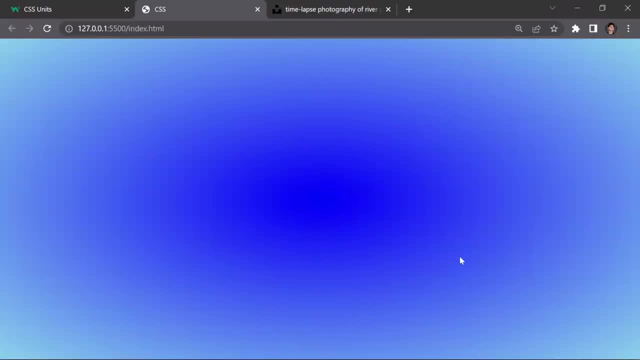 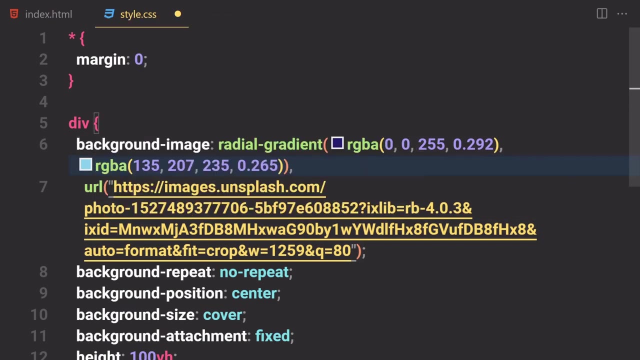 circular gradient and that linear gradient will gives us from top to bottom. okay, so if you want to change the opacity of it, you can also change the opacities, like. so. i'm going to change its capacities and save our file and this is how it looks like right now. 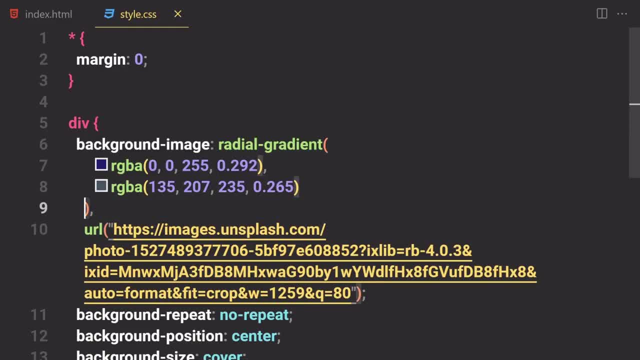 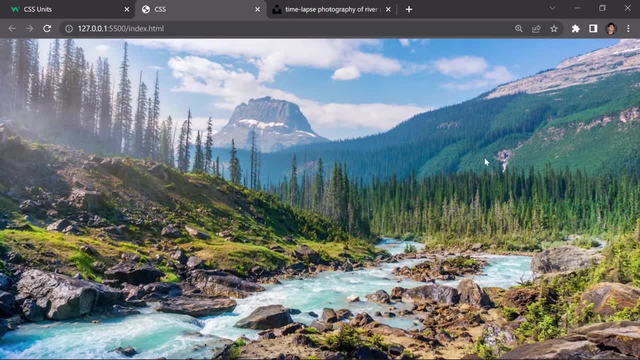 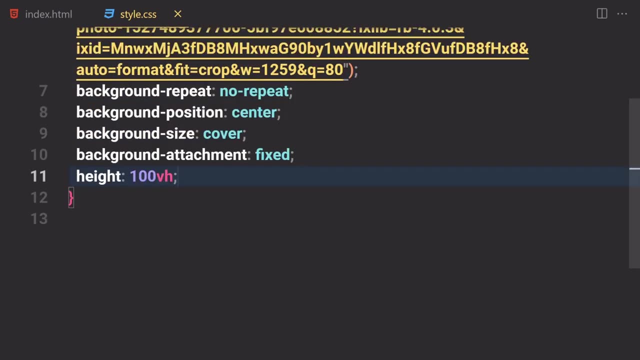 okay, and you can also apply that same values which i show you just a second ago to this image right here. so i'm going to just save that and this is how, by default, our image looks like. so now that we learn two kind of gradients, so we learn about a radial gradient and a linear. 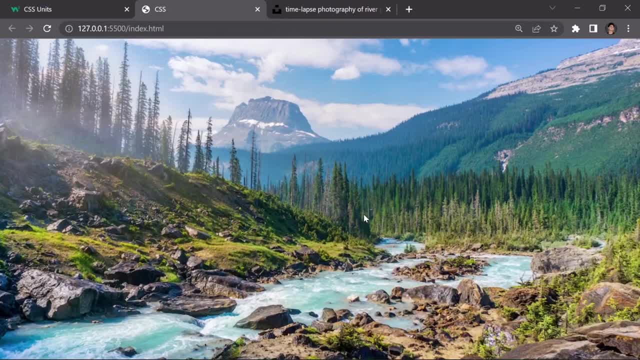 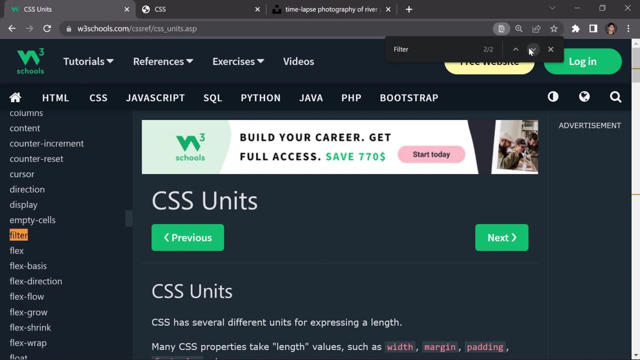 gradient. now let's learn about filters in css. so there are different kind of filters in css. so if you just search for like css filters and backdrop filter, and we have a filter- so i'm going to click on this one- and we have a gray scale. let me just show you that real quick. 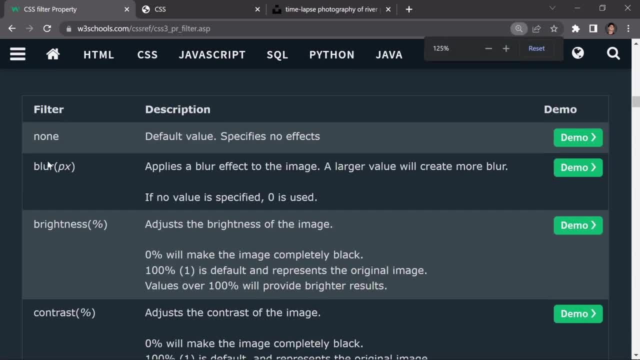 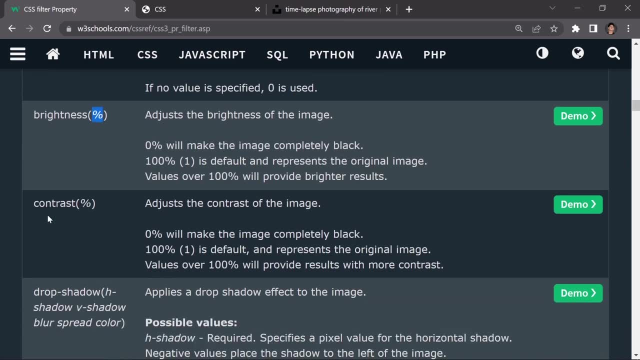 and these are kind of a new topics in css. so we have a blur. so, as the name suggested, we'll just blur our image and we can increase the brightness by using a percentage sign. we can increase their contrast by using a percentage sign. we can also work with a gray scale, hue and rotation, and in 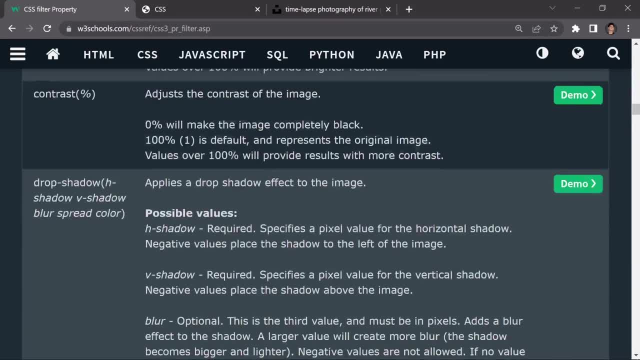 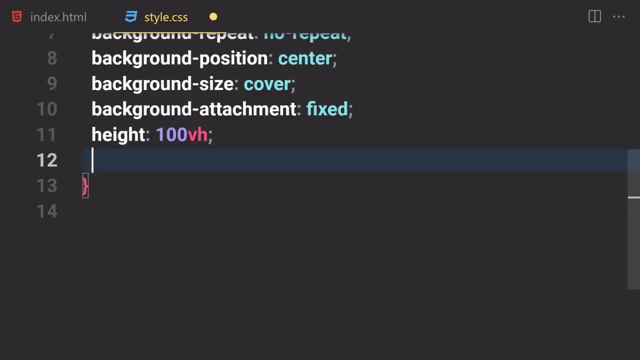 word- we can also work with opacity and so on and so forth. so, starting from the first thing, which is a blur, so if you want to provide a little bit of blurriness to this image, so for that we can use a filter and then blur. okay, so blur is a function which we can use, and here we have to specify the. 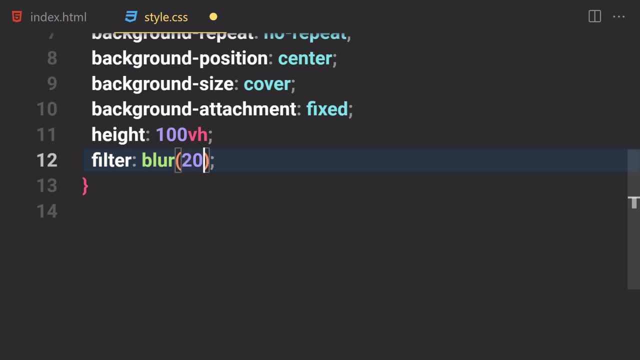 value like how much blur we want this image to be. so if you just want like 20 pixel, and if you save our file and here you can see, it will be now 20 pixel blur. if you want them to be like, uh, 60 or 60 pixels, so this is how our image will blur. if you want them to be like 10 pixel and maybe 5 pixel, 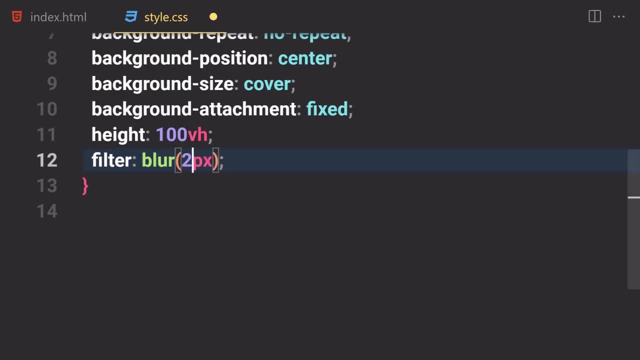 would be fine. and if you save that- and this is how a little bit blurriness can be show up right here- two pixel, one pixel, and so on and so forth, you can play around with that if you want to. in my case, i'm going to just stick to 10 pixel and i'm going to come to this line out. i'm going to write: 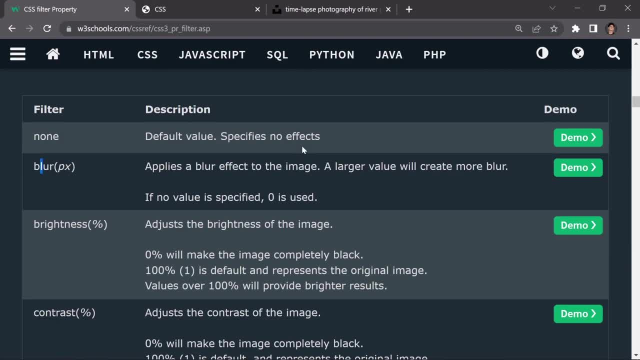 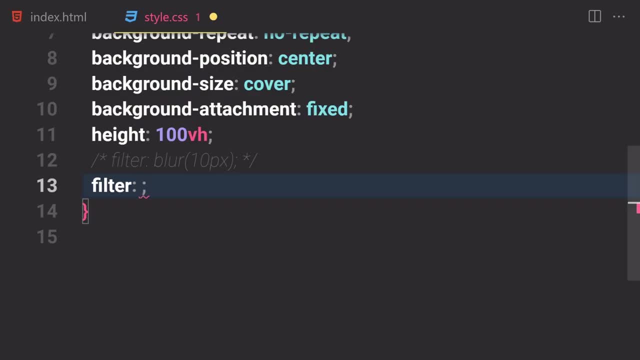 a filter one more time. and now the next property which i'm going to show you our the next uh function is a brightness. so as the name suggests that it will just increase or decrease the brightness of our image, so i'm going to just write like a brightness, and here we have to specify the 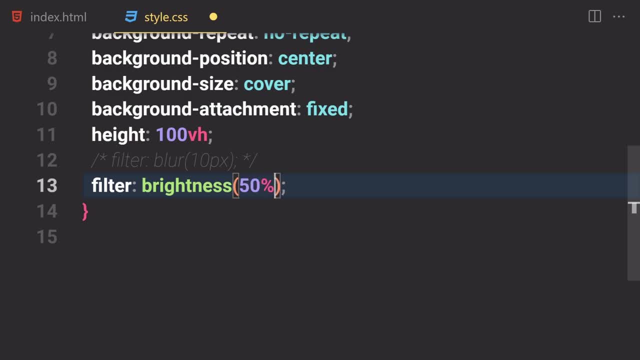 value in percentages. so i'm going to write like a 50 brightness. if you save that and here you can see kind of a dark, a night uh theme right here, that's because of 50 of that brightness. so if you want to get for like 100, so if you save that, so here you can see, it will now give us like by. 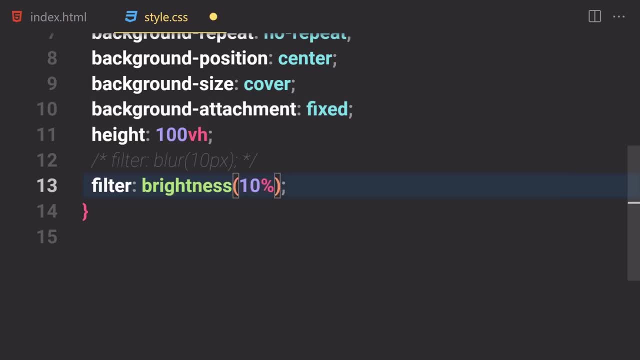 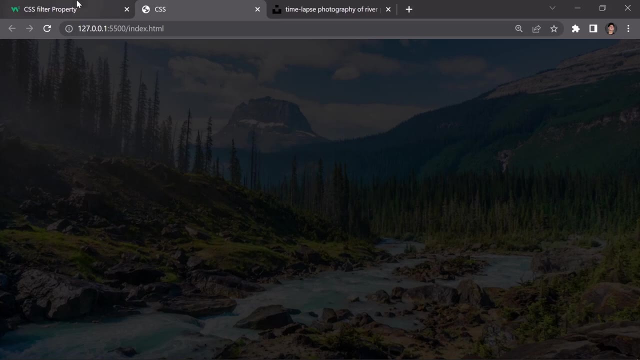 default image: uh, brightness. we can also work with the 10 value, so if you save that, it will be much more darker than the previous one. you can go like 41 and then 21, or and so on and so forth. so i'm going to just comment this line out and now let me write another filter and it will be. 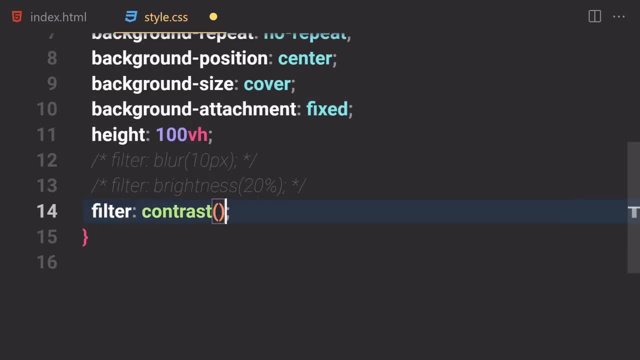 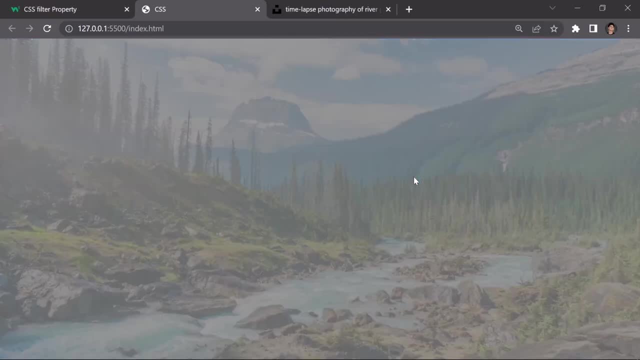 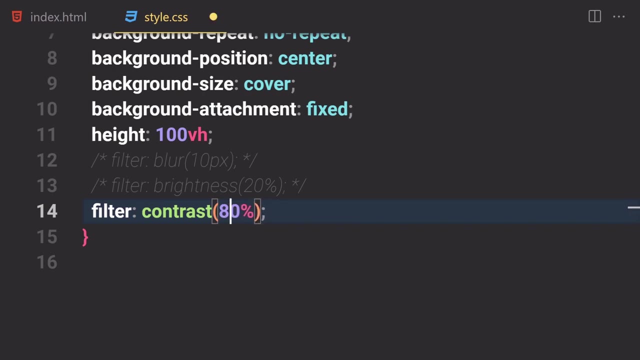 for contrast, as the name suggests that it will just increase the contrast. so if you just write like uh, first of all let me show you how our image will look like. this is our image if you want to increase the contrast. so 20 percent and 10 percent, or 100 or not thousand, but not 100. but you know. 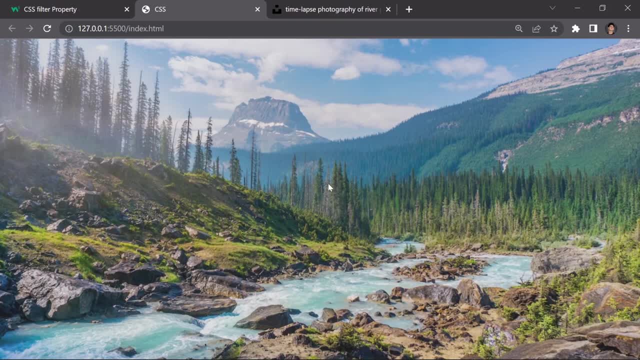 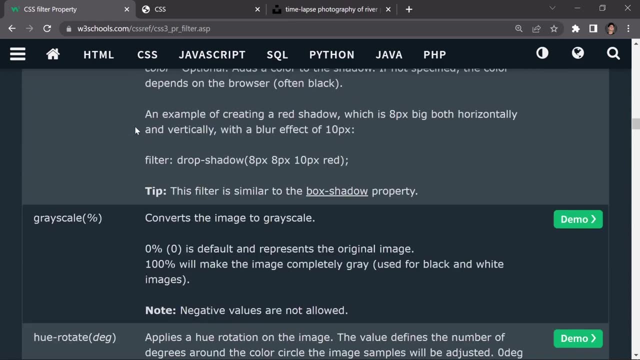 what eddie would be fine. seven, and this is how you can provide a contrast to it. okay, so now you don't have to worry about these drop shadow and stuff this kind of a little bit. oh, my goodness, there's a lot of talking. you don't have to worry about these drop shadows for now. you can use that if. 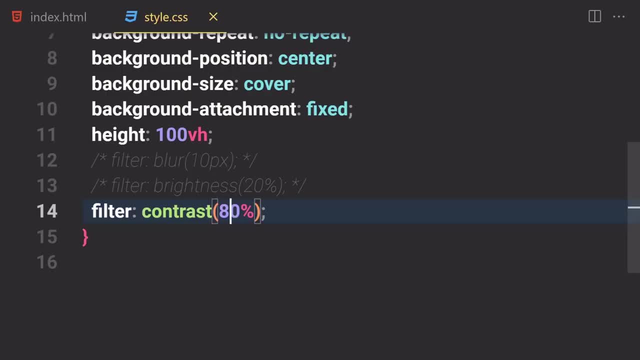 you want to. but now we will jump to the grayscale. so i'm going to comment this line out, and now let me just write a filter of grayscale, and here i'm going to just provide like 20 percent. so if you save that, so you cannot see something. uh, you know, i'm going to write like one percent, you can still. 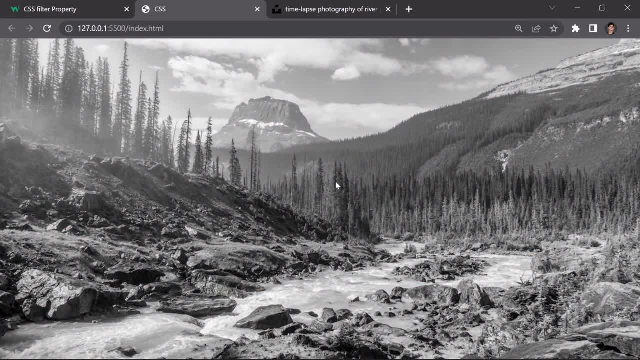 see that there. so if you're at 100 percent, so here you can see it will not increase the contrast, but i'm going to make it black and white. that's because of a grayscale function. okay, so we can provide like a 70 percent. so this will be the 70 percent. kind of old school, low quality images. 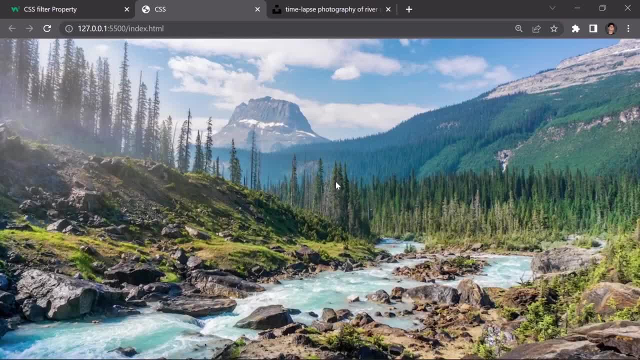 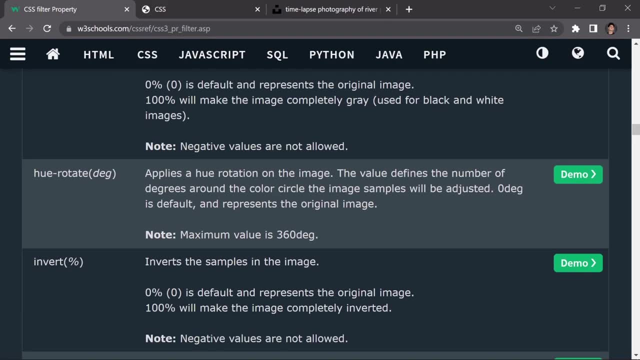 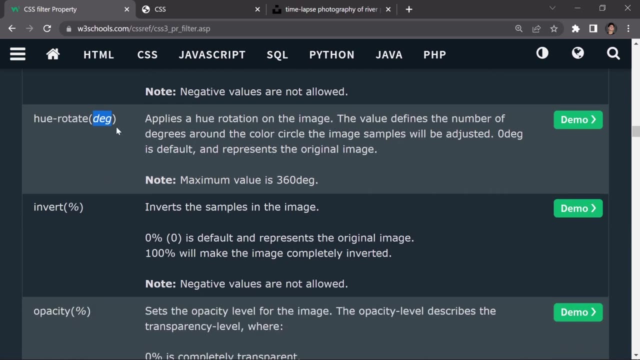 we can provide 40 percent, and i guess that 10 would be the default one, or we can just remove that, and this is how it looks like. okay, so we have gray scale, we have a hue and rotation, and here we have to provide a degree, and we will learn about a degree. deg is also just a unit which allows us to 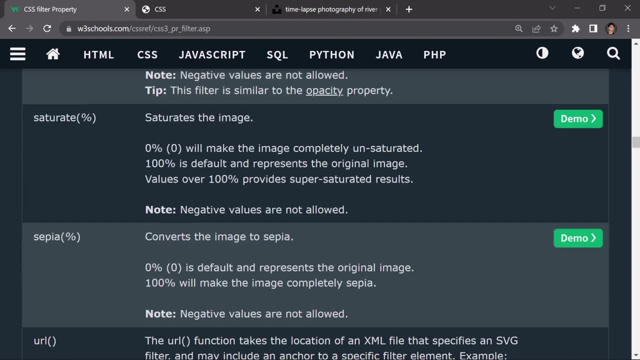 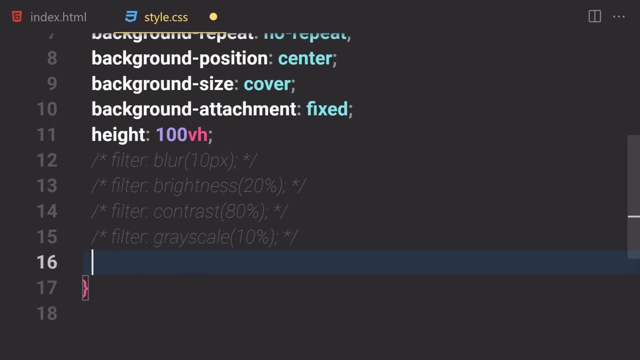 we can provide inversion, like in word or opacity saturation, or you know what? i'm going to just show you this saturation and you can explore the other one by yourself. i don't want to waste your time, and mine as well, so here i'm going to just write a saturation of. maybe let me just write a 40. 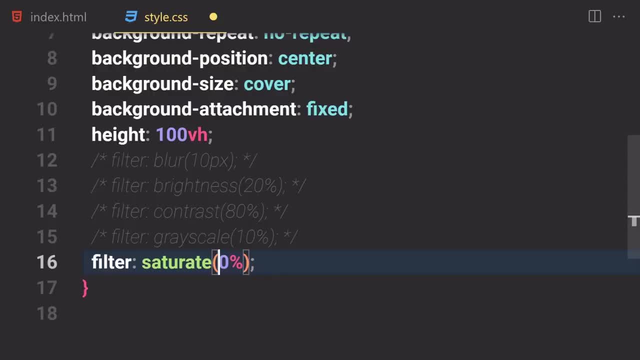 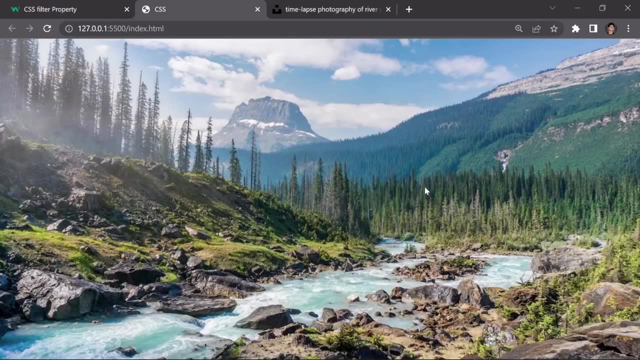 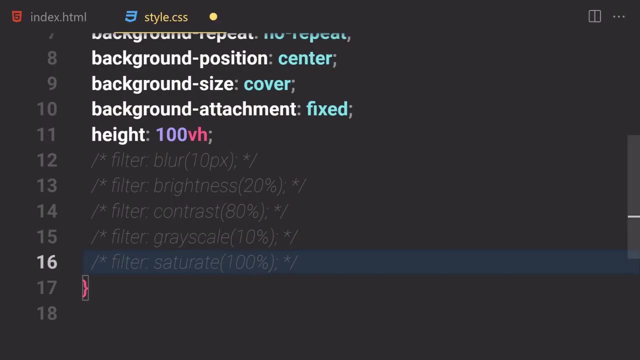 percent, save it. and this is looking a bit kind of a black and white. let me just write- uh, i don't know- 60, a little bit more kind of a greeny. let me just write 80, a little bit more green. so 30 percent will be just a high quality of saturation. so you can play around with that if 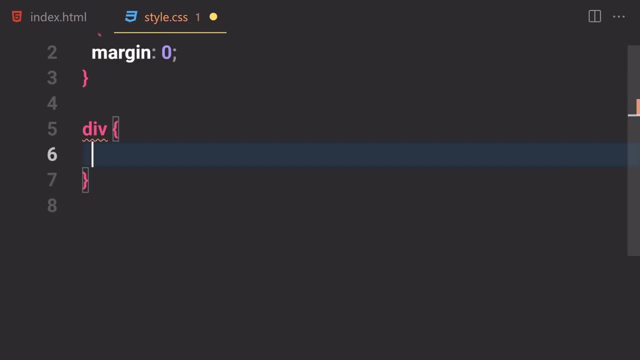 you want to, but for me, i'm totally done by showing you gradients and filters in this video. so i'm going to remove this div, i'm going to also remove that dev and boom, everything is gone, all right. so now that we learned enough about gradient and filters, so now let me just show. 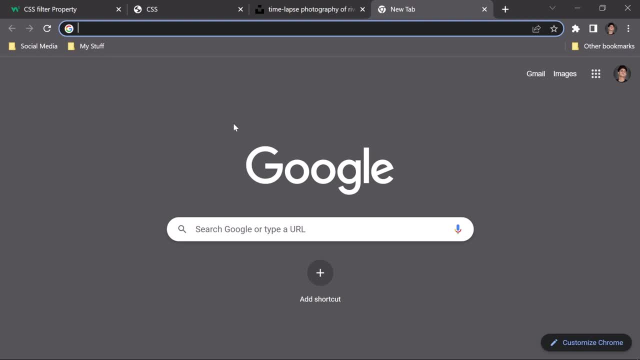 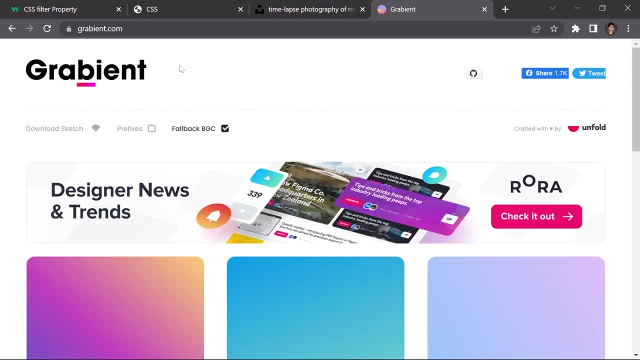 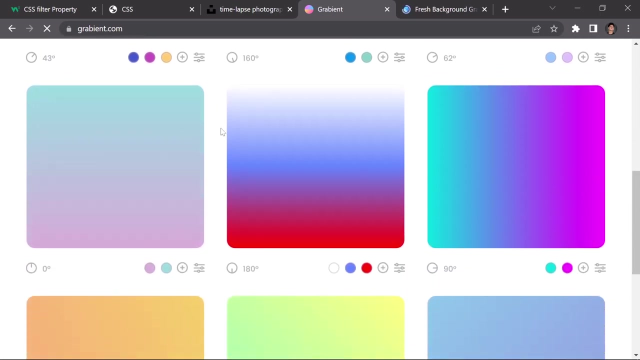 you a cool places to find a gradient for yourself. so the first place i will show you is something called a gradientio- not gradientio, but just a gradientcom- and the second place i'm going to show you is web gradientcom. okay, so these are the places where you can find a lot of great gradients for your. 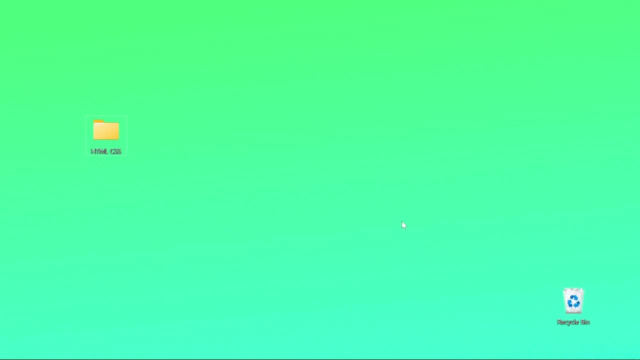 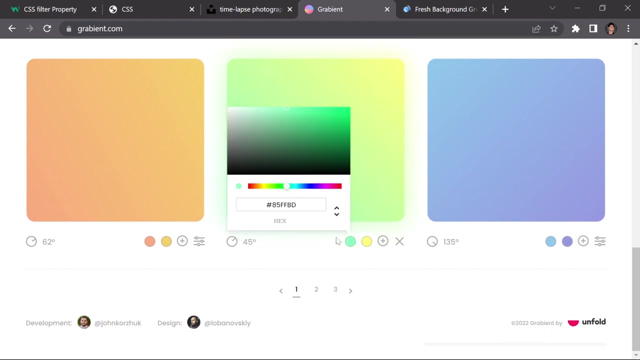 project. so i just choose, like i guess i choose this gradient from this website somewhere i don't know. but if you want to just work with that gradient, so you can just click on that and you can copy this hex code and put it inside your gradient. and you can copy that one and put it. 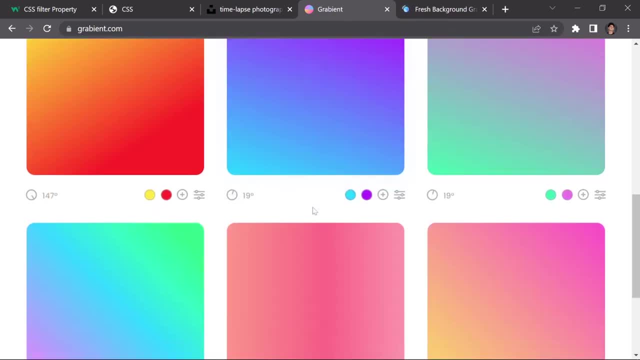 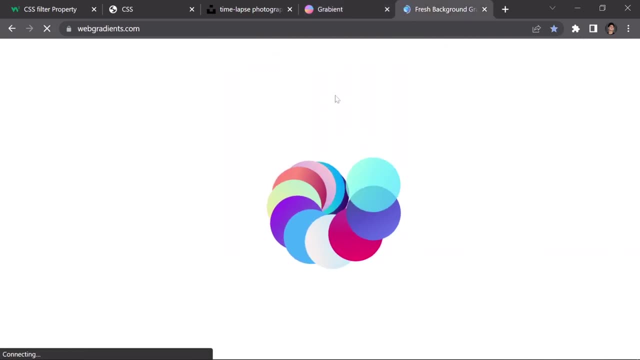 inside your project. okay, so we have like three pages. this is the second page and this one is now the third page right here. okay, so this is the first website, right here and now. this is the best way to find a gradient for your project. so now let me just show you that real quick. here you: 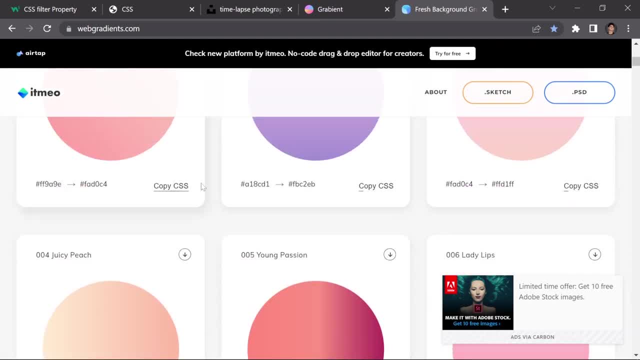 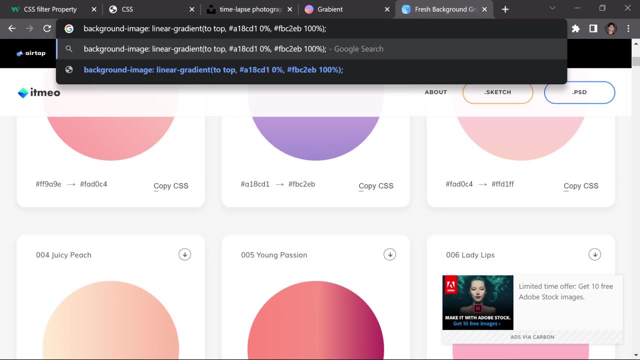 can see a lot of cool gradients. you can copy the css code you want. so if i just click on that, let's suppose, and if i just pass it right here, so it will like use this like background image of linear gradient to top and then the first color, and then it will also give you these percentages. 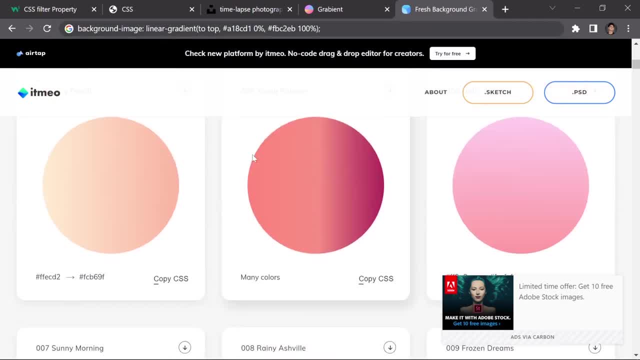 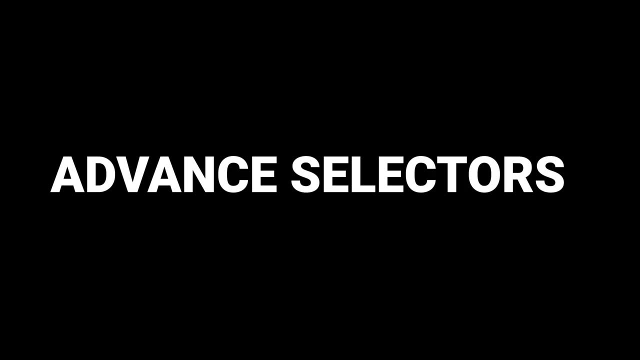 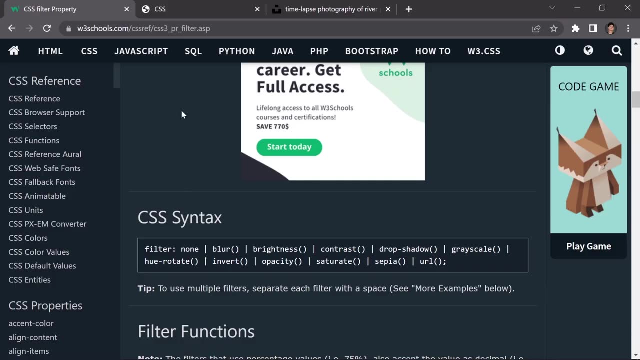 and then the second color and its percentages as well. okay, so you can choose a lot of gradients from this side. okay, so that's what i want to show you now. the next thing which we are going to be learning about in css is something called selector. so so far, we've been using this selector like if. 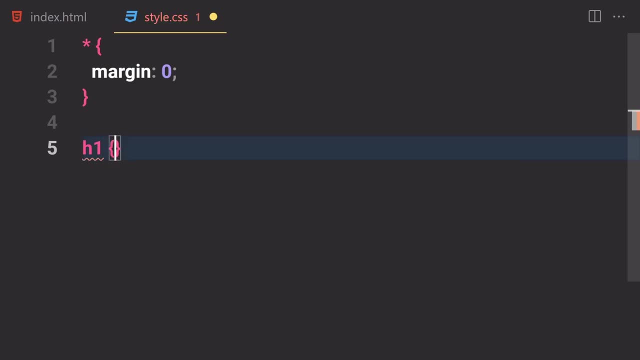 you want to select something by using, uh, css, so we just first of all write the selector name like a tag name and then we just write our stuff inside the css. but this is just a little bit of a one way to select some. but if you want to work with a real world project, so for that we are. 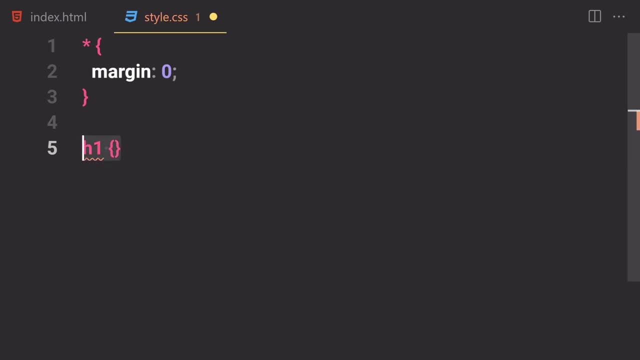 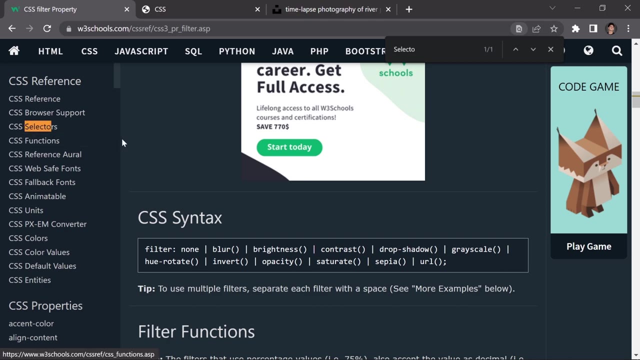 going to be using a lot of selectors, so this is what we are going to be learning in this section. so now, if you just ask for a girlfriend like w3 school and if you just search for uh selectors here, you can see we have this css selector. so if i click on that, and what brings us to this page? 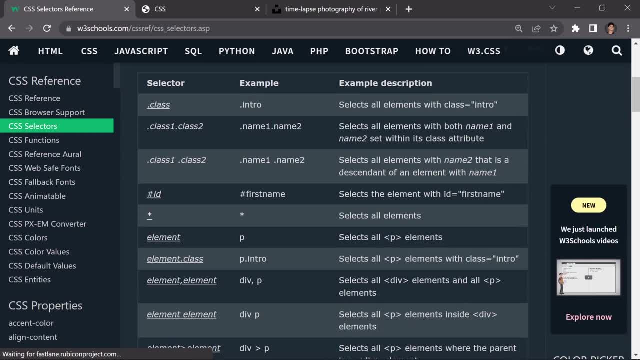 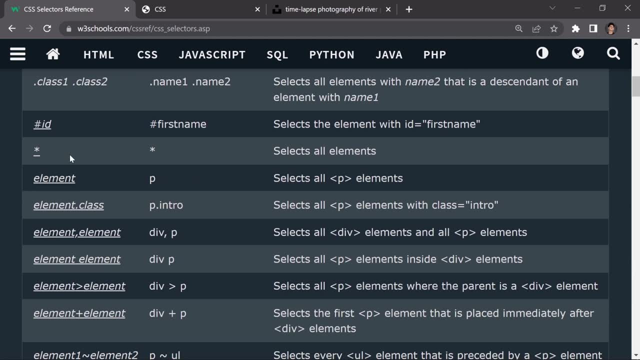 right here and there are like crazy amount of selector but we would just need a few of them. we have a class selector, double class selector or multiple class selector, or you want to call it. then we have id selector, everything selector, just a paragraph selector, paragraph with the intro, intro class on it, every paragraph inside. 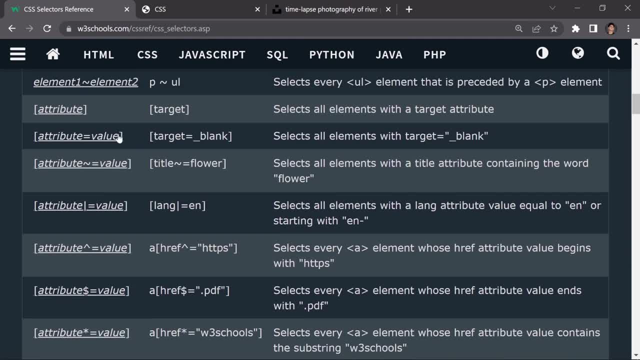 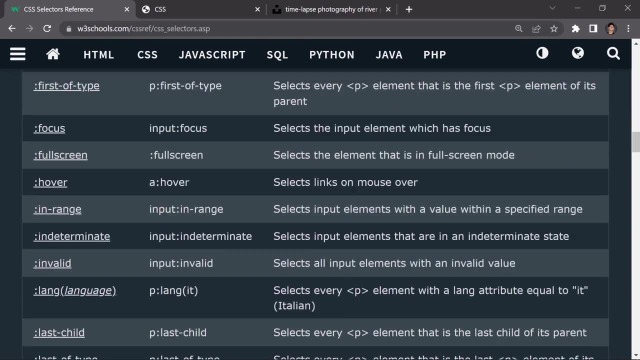 the dev and we have like crazy amount of css selectors, we have attribute selectors and these are something called um pseudo selector, which we are going to be also learning, but not in this video. okay, so starting from the first one, which is a class selector, so if you want to select, 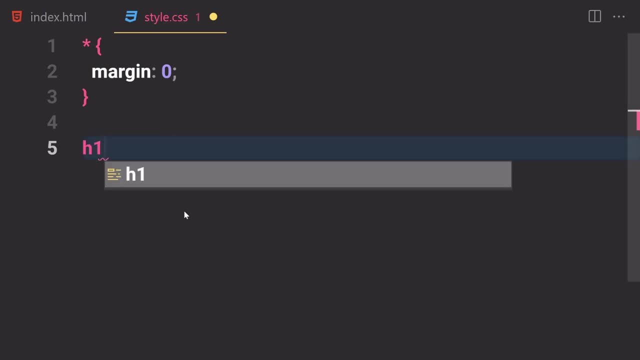 something in css. so the first way we already saw is that first of all, just write a selector name like a tag name, and then just try it. or opening curly brace and then closing curly brace. but now, in this case, let me just remove everything from this document. and now, in this case, let's. 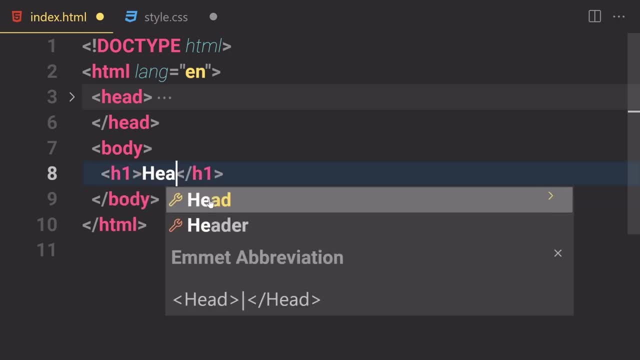 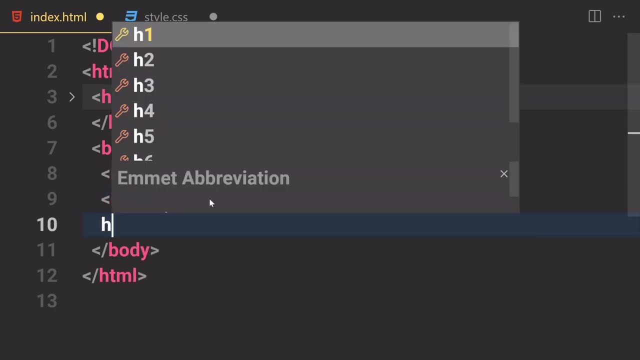 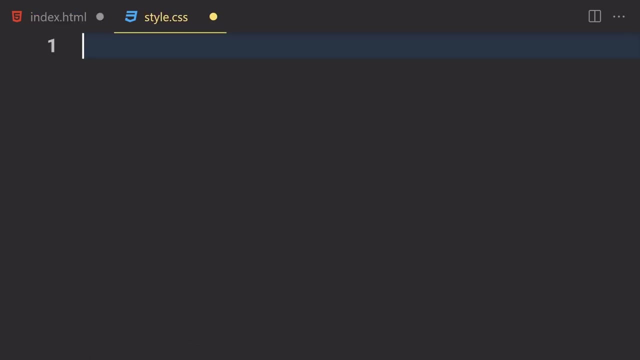 suppose if you have like multiple thing, if i want to select like h1 and we have heading uh one, then we have like h2 of heading two, then we have like h3 of heading three. suppose if you want to select this h2 by not using the tag name, like we don't want to select there by using h2, and then want 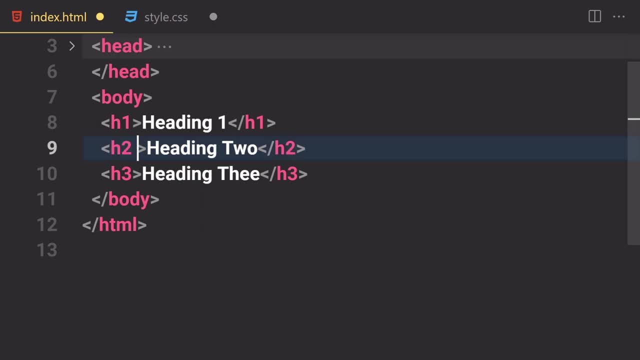 to work with that. so the next way we can do is that we have to provide a class owner. so now, if we want to write a class to it, so first of all we are going to be writing a space and then we will just write a class and we can give like as many classes as we want right here. okay, but if you want, 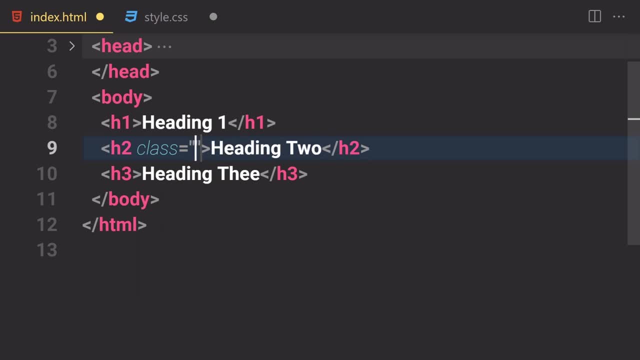 to separate two classes from one, so for that we are going to have to just provide a space in there. okay, so now let's suppose, if you want to give him like two classes, like one, and i want to give him another, so for that we have to write a space, and then we can write two, three, four, and how many. 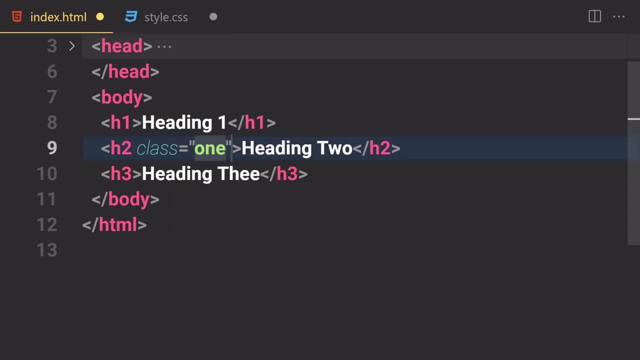 classes you like. okay, so now, in this case, we want to just select this by using a class selector, so to provide a class right here, like class attribute to be precise. so now, if you want to select that in css, so what do we have to do? first of all, we have to- let me just save this file. first of all, we have 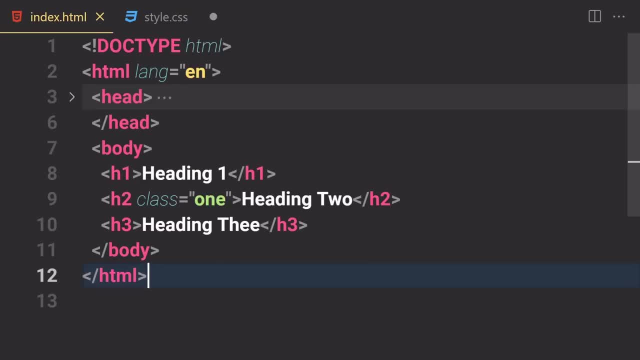 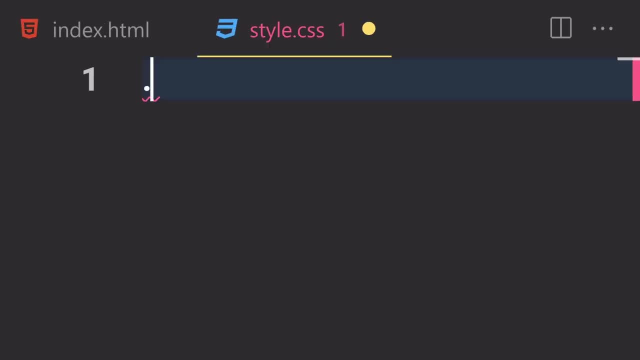 to go towards css. and now, if you want to select this class like one, so for that we have to first of all write a period, or dot, whatever you want to call it. let me just zoom in a bit so you guys can see everything a bit better. so first of all we have to write this period and then the class name. 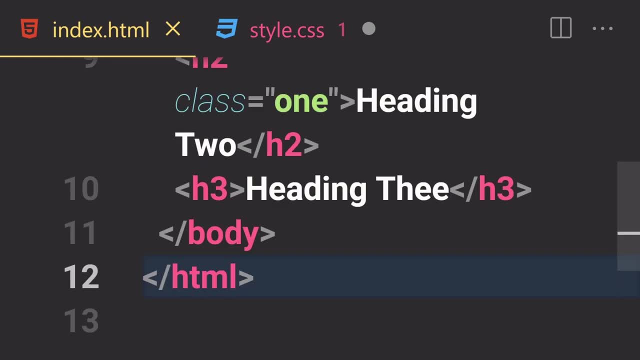 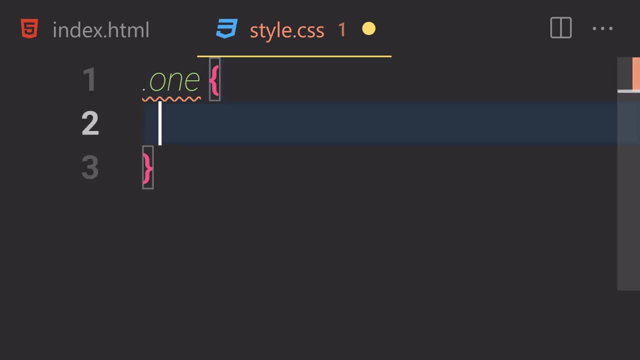 so what is the class name? the class name is just simple one, so we have to just write one here and then opening curly brace and then closing curly brace, right here and now. if i hit enter now, i can do whatever i want to do with that. suppose. if i want to change the color to be like maybe. 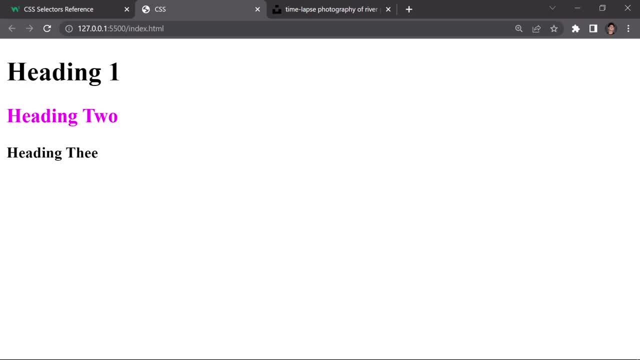 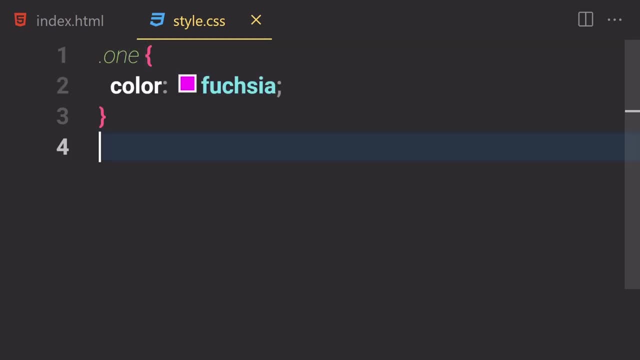 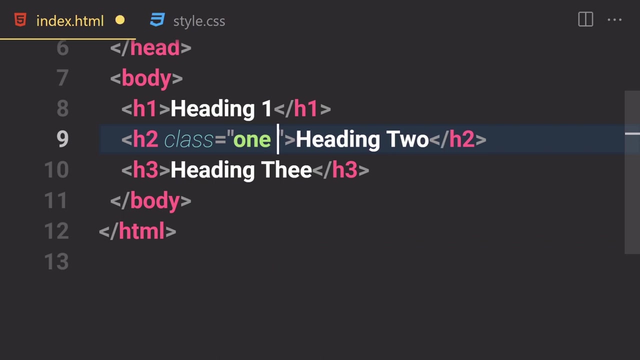 fuchsia, and if i save my file and go to my css, so here you can see, it unlock uses like fuchsia color right here. so this is how we can select everything by using classes. so now let me just show you a multiple classes. so if you just provide a cluster, it's like one, and we also want to provide, uh like 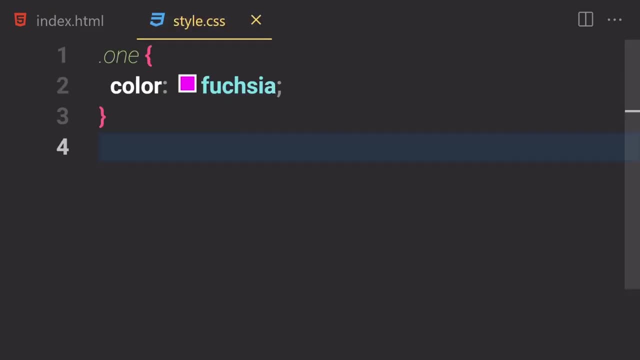 two class. so now, if we save that, we can also do that right here. so let me just select this two. so it will provide this uh styling as well, because we have this class available inside this heading right here, like we have one class available inside this h2, so it will provide this. 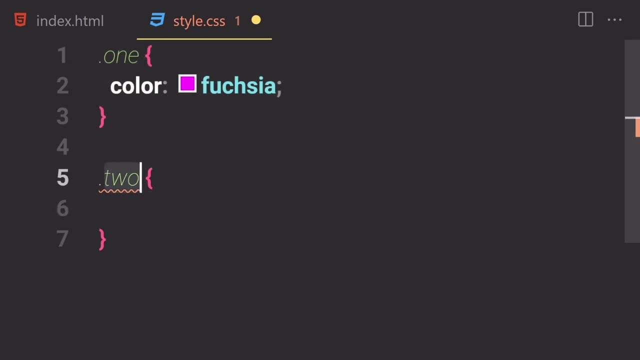 styling as well. and now if you write some more styling in this two class, so it will also apply there, because we have these two classes as well. so let me just write something like i don't know, maybe i'll just increase the font size to be like uh 4 ram, and if you save that and boom. 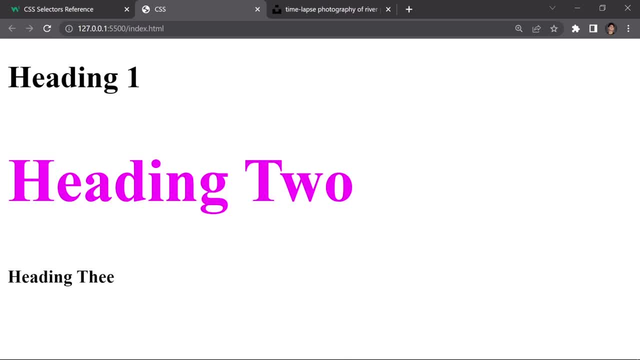 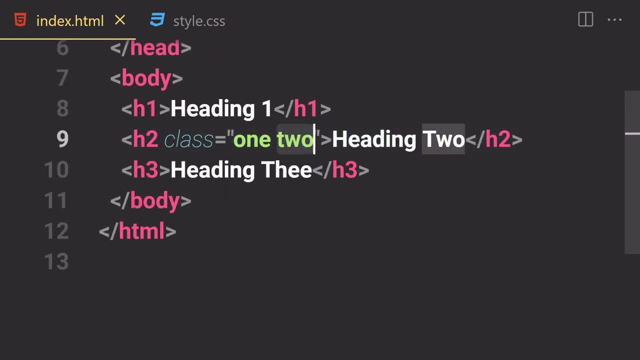 here, you can see. it will now also increase the font size to be, uh, four rams right here. okay, so now if i just forgot to include this second class, or if i didn't include this second closing, and now if you just remove that in some case, so now let me just save my. 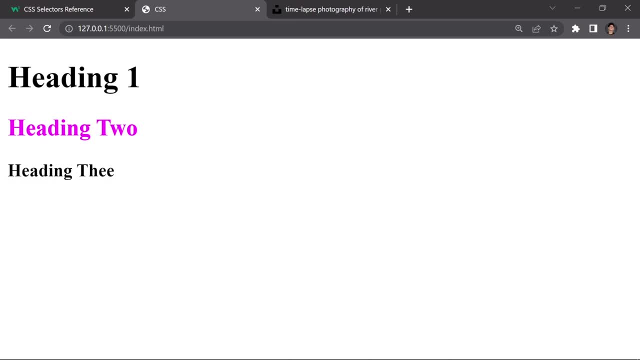 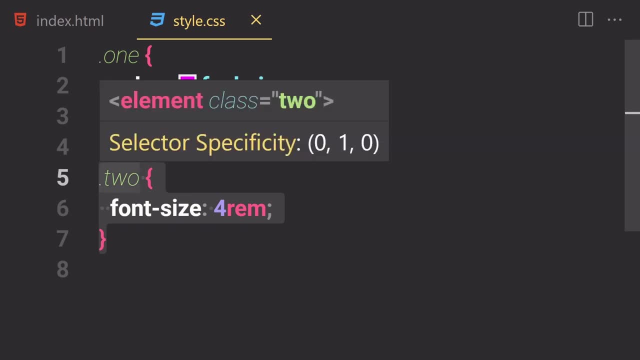 file and here you can see it will change the color but it will not change the font size of it. that is because we don't provide, uh, that styling to it. we did declare our styling inside this second or two, to be precise these two claws, but we didn't use this two clause somewhere inside. 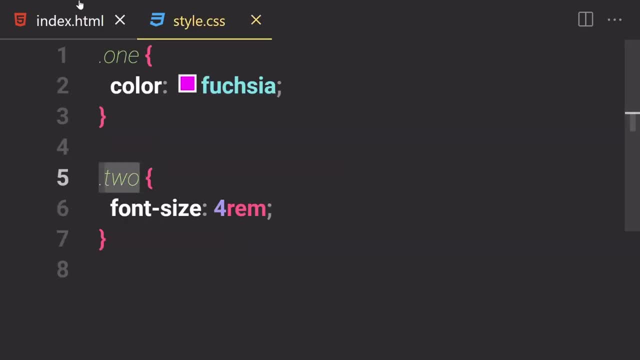 word css. if you are using it right now, i'll teach you how to use it like this: just opening one and down, going in and courageousing going in, going in. it will open it up. it will change the font size. but if i want to use this class like this two class inside this h3, we can also do this. now let me. 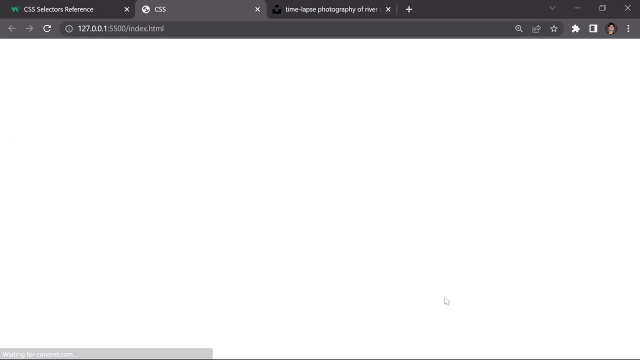 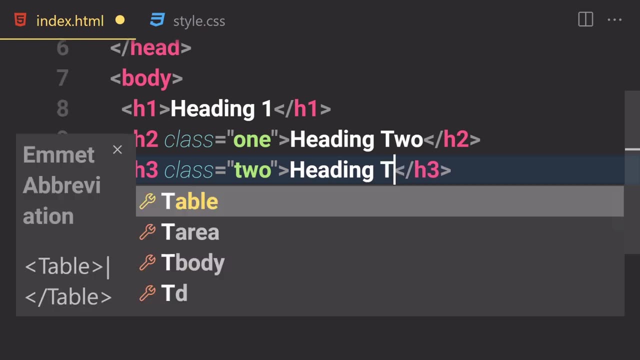 just write a class in here, and now let me just write two. and now if i save that and boom, here you can see it will now just increase the font size of it. and i just realized that i made a mistake of uh, th, r, w, e, three or three, so three. so now, if you save that, and now it's looking better. 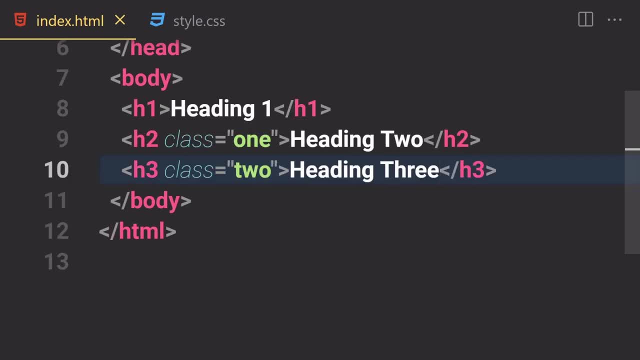 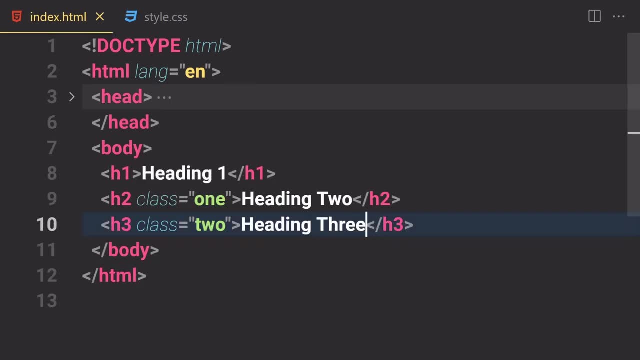 so now you are getting the idea of classes. so this is how we can select everything by using the classes. okay, so i guess i bump it up a lot. let me just zoom out a bit so you guys can see everything a bit clear. so we can select something by your tag name and. 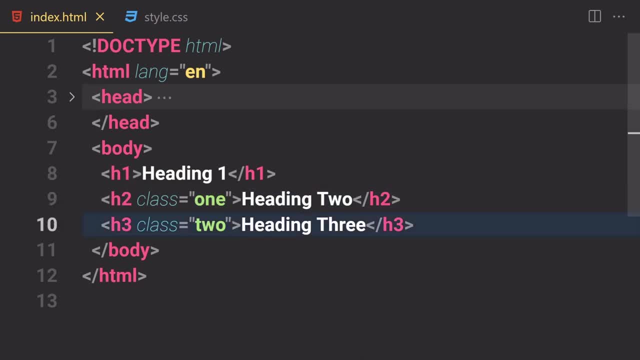 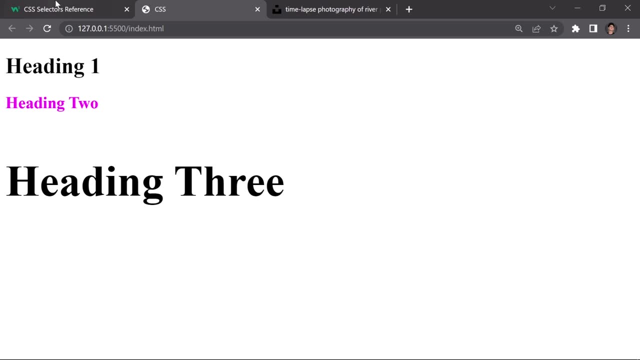 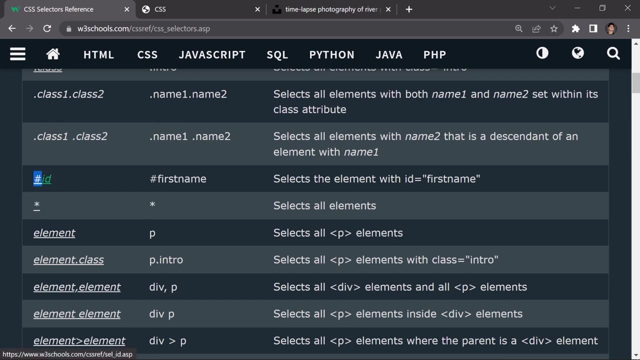 we can also select something by using classes, so we can provide multiple classes, but we cannot provide multiple ids to one element. so what are ids? now, let's just learn about that. if you want to select something by using id, so first of all you just have to write a pound symbol and then. 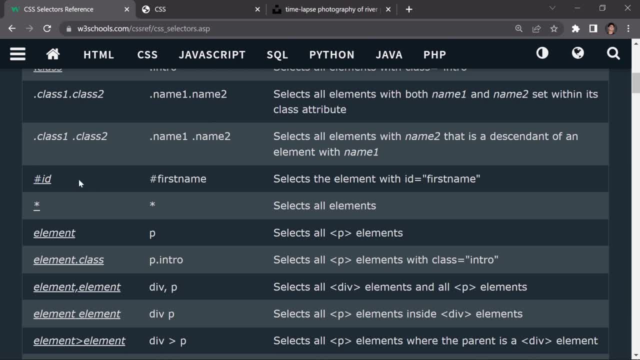 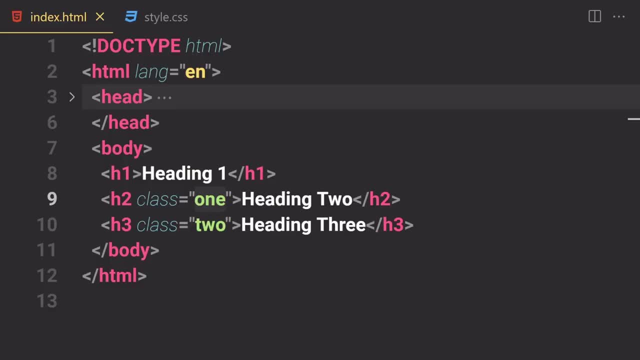 first of all you have to give them some sort of id to your animal element and then, if you want to select that element by using a css, so first of all you have to provide a pound symbol and then the id name. so first of all let me just write some code then. 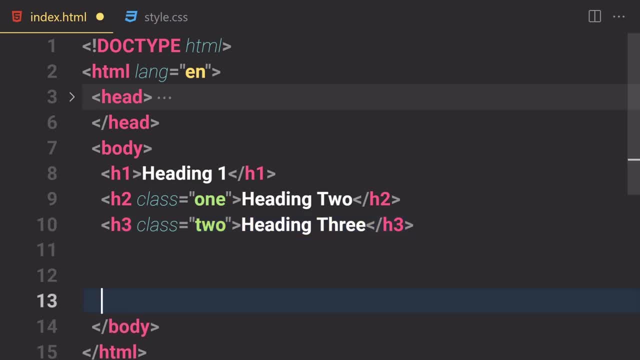 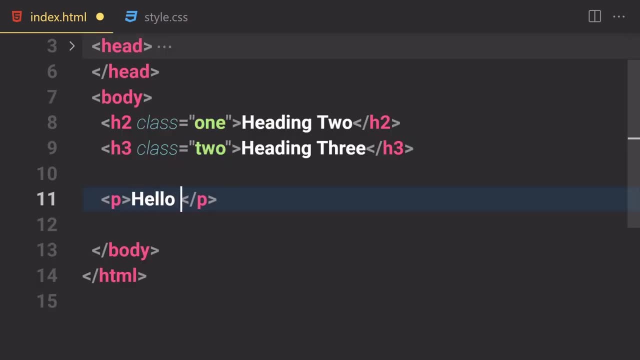 you'll get to know what i'm talking about. so now you know what i'm going to just write. i'm going to remove this h1 from here and here. i'm going to write a paragraph right here and i'm going to just write like: hello, i am id selector, or just id would be fine. and now if i want to give him id, so what? 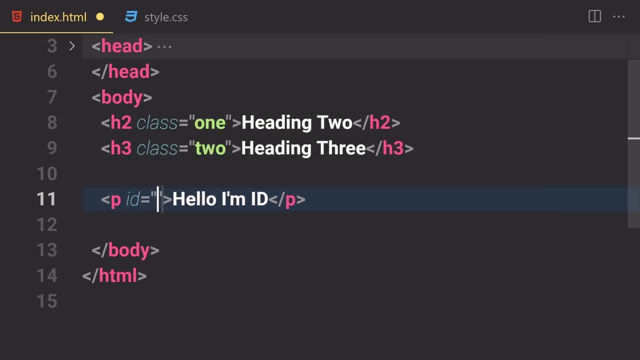 do i have to do? i just have to write id and if i hit tab so it will now give us like. it will not auto complete for us, so here we can provide like: uh, id and ids are special in css. you have to remember that the ids are totally special. you cannot put like two ids if i want to just write. 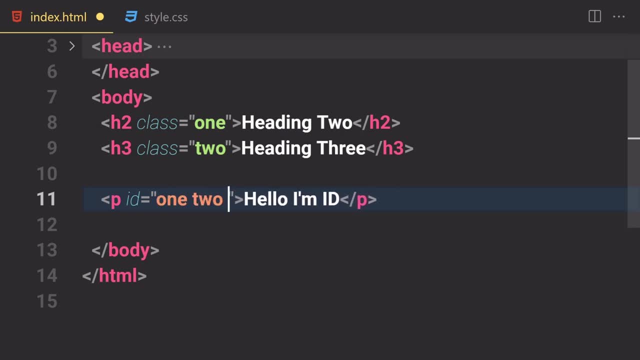 like one and then two and then three, so it will not work. both of them will not work. ids are special, so you have to use id once. you can reuse this styling again and again, but you cannot provide two ids like id will be one. you can reuse this styling again and again, but you cannot provide two ids like id will be one. 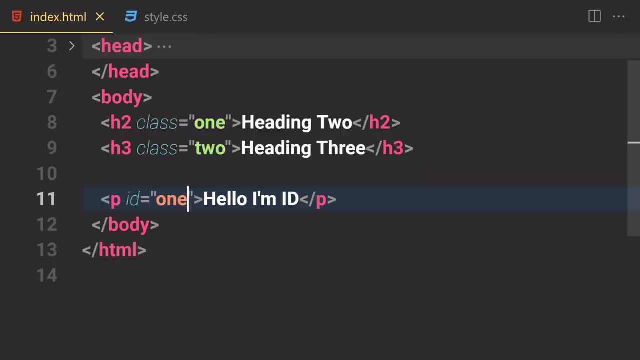 you can reuse this styling again and again, but you cannot provide two ids like id will be one, okay, so now, if you save that and now here you can see, nothing will happen because we do declare or id right here, but we didn't provide any styling to it. so if you want to provide a styling to it, 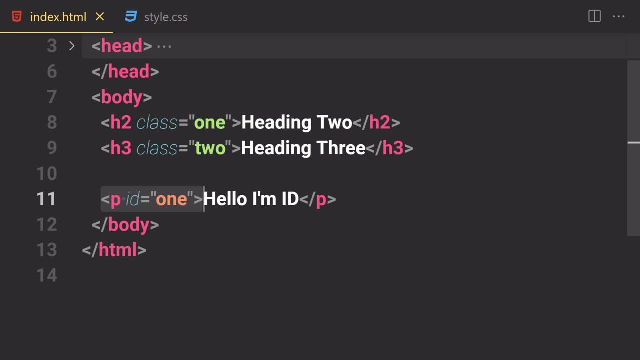 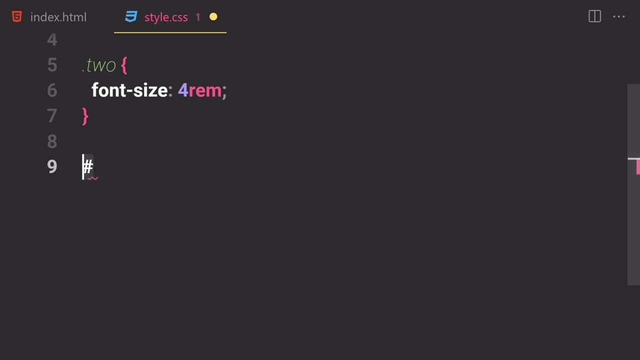 or, first of all, if you want to select this paragraph by using this id. so how can you do that? well, you just have to go to your css and first of all, you just have to write this pound symbol or hash symbol, whatever you want to call it, and then the id name. so what was the id name? the id name. 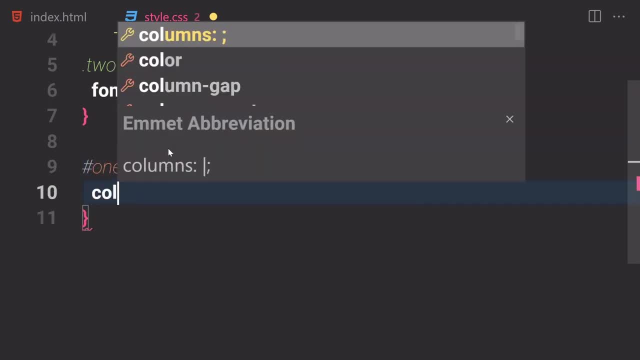 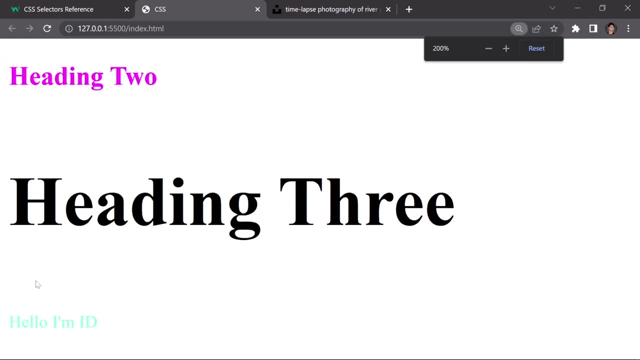 was just one. so now you just select that and here we can just provide different kind of styles or whatever we have like. let's suppose i'm gonna just provide this color and now if you save that and here you can see the colors change to this kind of color, like a greenish color. okay, so if i 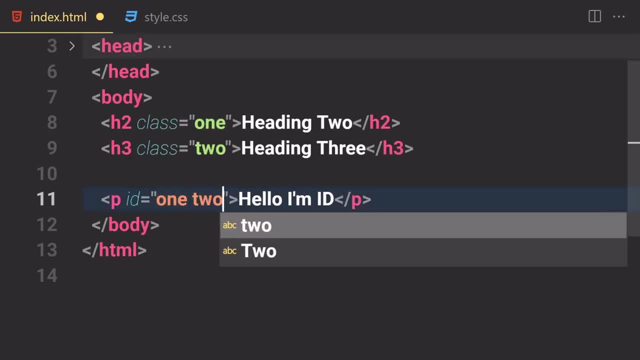 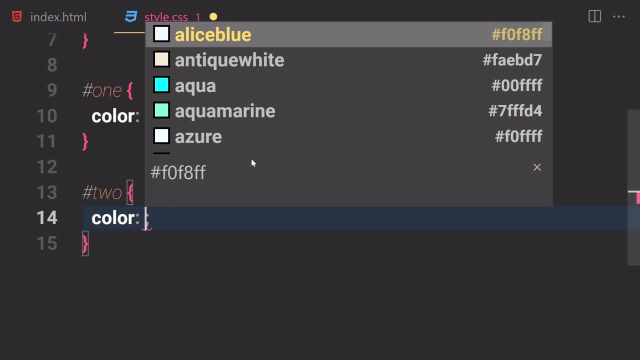 try to provide another class. uh, i mean like id. so let's just write like two and save our file. and now let me just uh, select my second id right here and now let me just provide a color of, or you know what. instead of color, i'm going to just increase the font size to be like four ram. and now, if you, 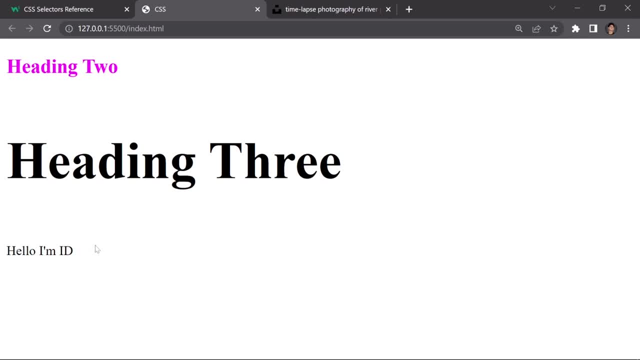 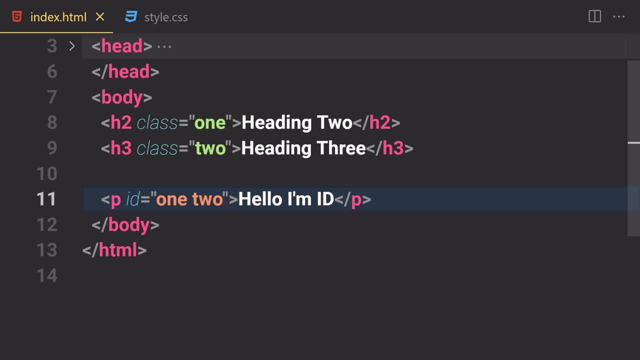 save that. and here you can see it will not increase the font size. why? because, as i said, that ids are special in css and you can provide just only one id to your um, to your element. okay, so i'm going to just remove that. i'm going to totally remove this paragraph and also these. 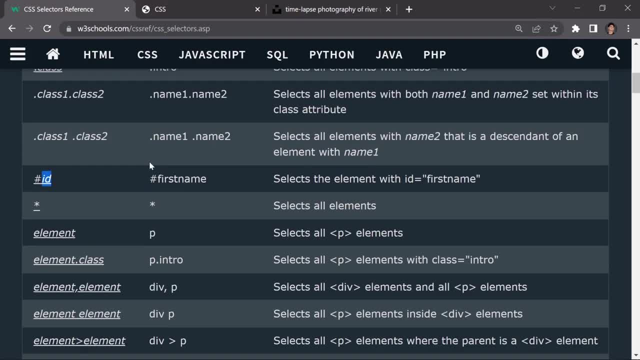 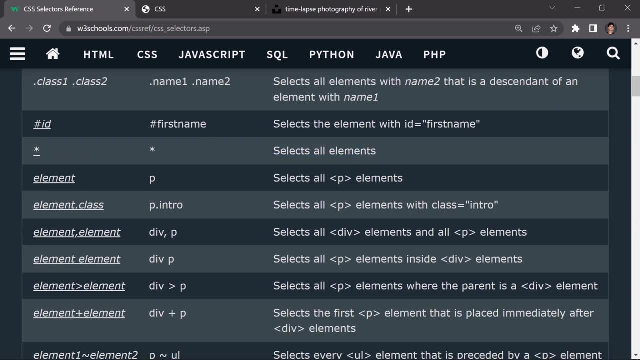 classes as well. so now let's jump into another css selector, which is called an everything selector. so, as the name suggests that it will be like everything selector, it allows us to select everything, and this is known as a asterisk, or whatever you want to call it. so now, if i didn't 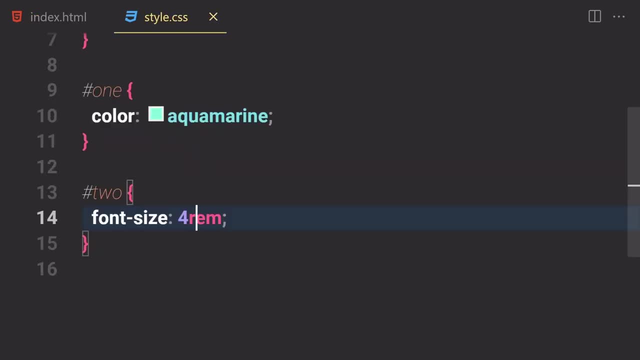 write anything inside a body. so if i save this file and then i'll just select everything and i'll go to my css and i'm going to remove everything from it, and then if i want to select everything, like if i want to select my uh, html head, title, body or whatever we have, so we can. 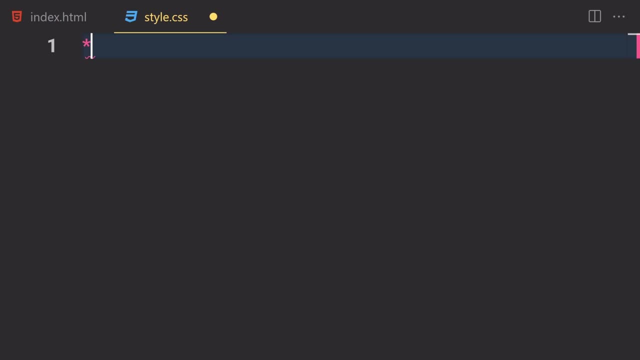 just write this asterisk symbol. so you just have to first of all hold shift and then hit add, so it will now give us this symbol right here and now, if you want to, just writing a style like border of two pixels, solid red, and now if you save that, and now if you go toward css. and now, here you can. 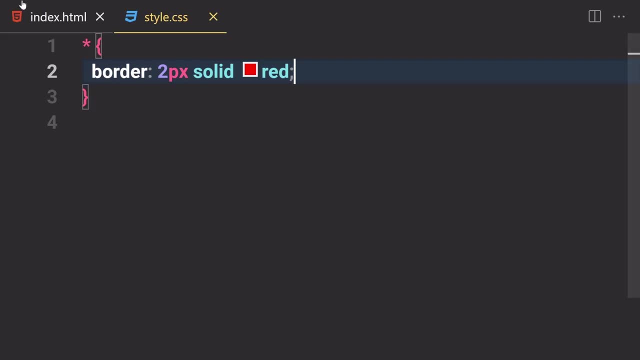 see. now you might be asking: like where is this style coming from? like we didn't write anything inside this body tag. that's because it is selecting- uh, what do we call it? head area and the html area and also the body area. so if i type something like h1 of, like hello, and now if you save that, so here, 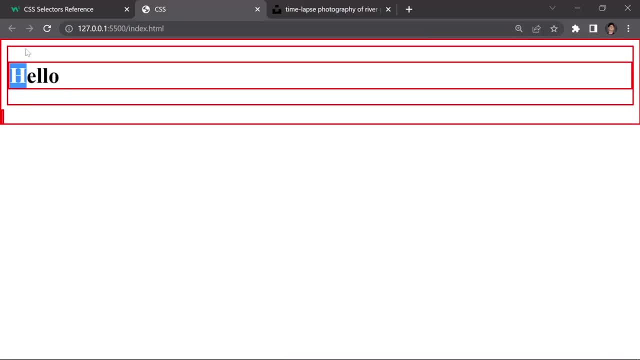 you can see, it will also select there. it will provide a border of uh, red right here. if i write like span in some case, like in my case, i'll just write like world maybe, and now, if you save that, it will also select this span and it will provide this border to it. okay, so this is known as 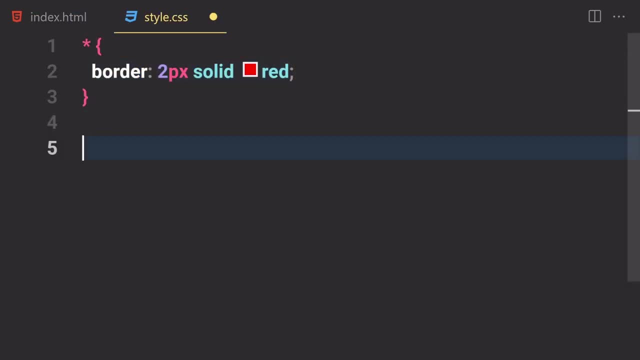 everything selector and it will select everything. it can be very handy in some situation, like in some situation we would have a section and let me just write a section, and then we would have like i don't know article maybe, and then we have like, uh, i don't know main, okay, so we would have a little bit of content inside there, like one, two. 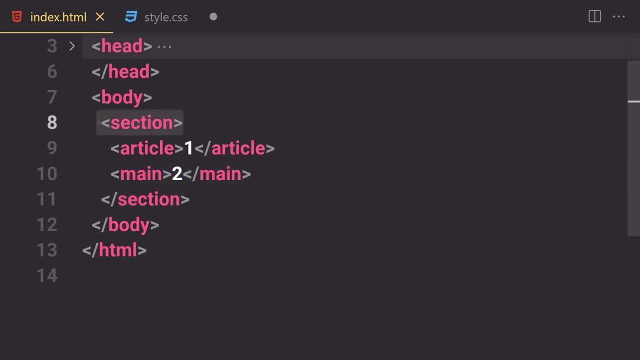 and so on and so forth. if you want to select everything which is inside this section area, like you have maybe a 500 line of code and you want to select all of that, so for that you can use: just first of all write a section and then just write everything- selector. now let me just 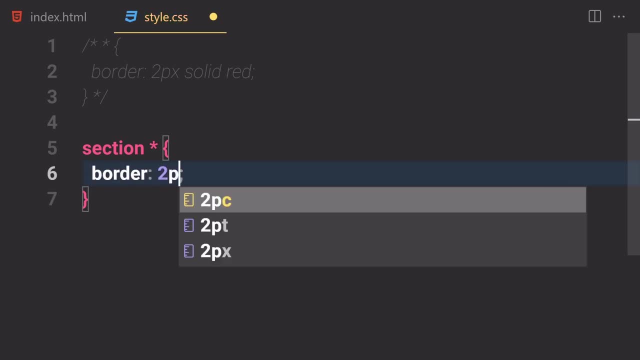 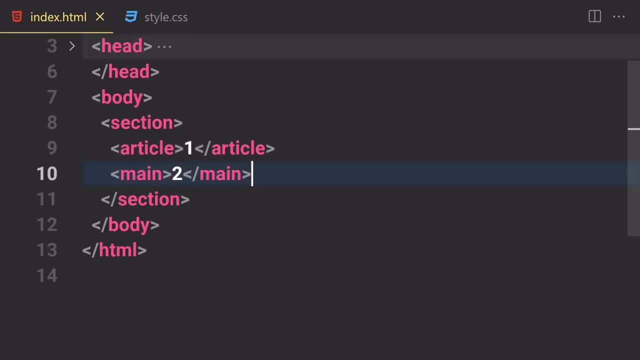 comment there for a second, and here i'm going to just write like a border of two pixels solid teal, and now, if you save that, and now here you can see, it will now select both of these items which we wrote right here. okay, if you just write like i don't know, h2 of um, maybe three, and if you save, 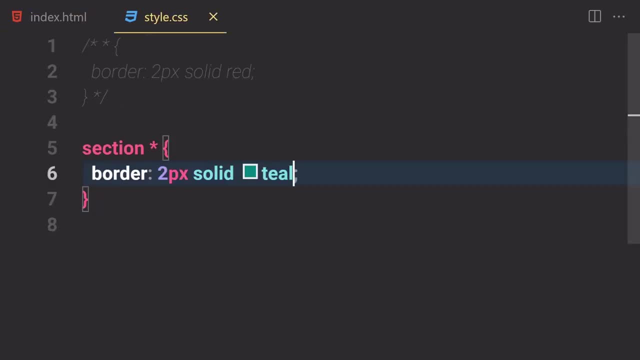 that, so it will also select this one as well. okay, so these everything selected- can be very helpful in different kind of situations. so now i'm going to remove everything from css and everything from a body as well. okay, now the next selector which we are going to be talking is just: 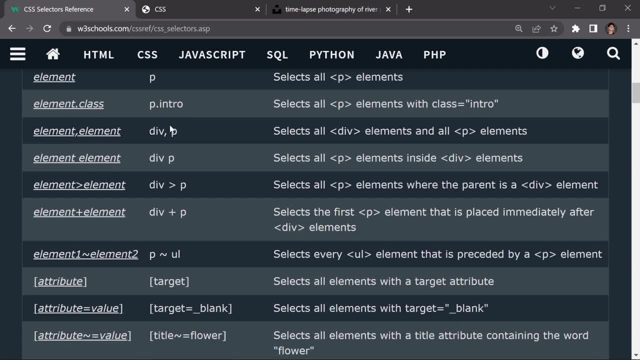 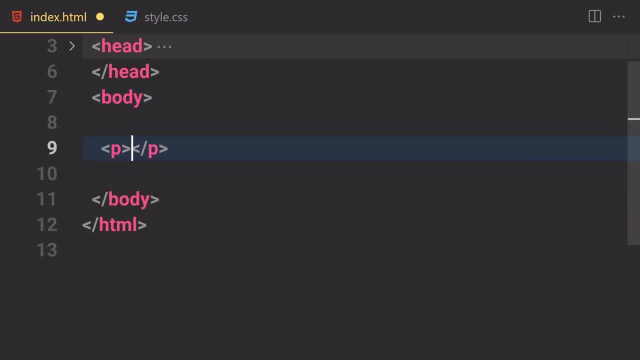 an element selector, which you already know how to select something by using an element selector, you can also provide a specific clause to it. so let's suppose we have two paragraph. suppose you have a paragraph of hello and then you have a div and inside this div we have a p and we give them a. 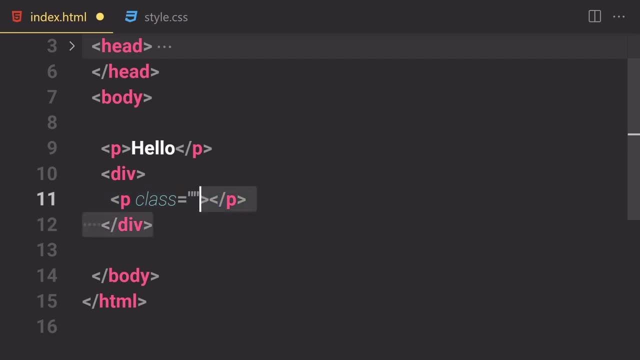 class of um. you know what? i'm not going to providing any classes, but i'll just write a div and i'm going to write hello inside there. and now, what i'll do is that i'll just specifically provide a cluster like um. i'm going to just write like: 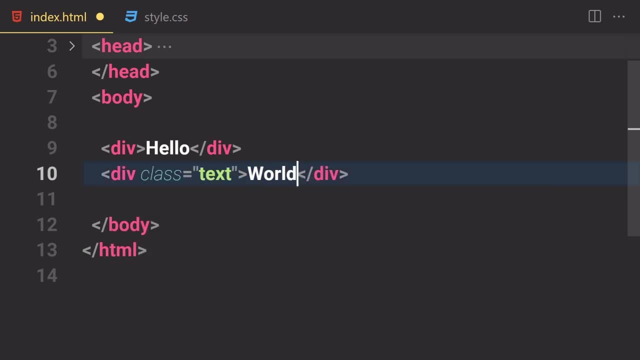 text or content would be fine, and i'm going to just write like world inside there. so now this div doesn't have any classes. this div do have class. so now, if you want to specifically select that, so for that we just have to write div with the class of text. do you just provide a text? yeah, 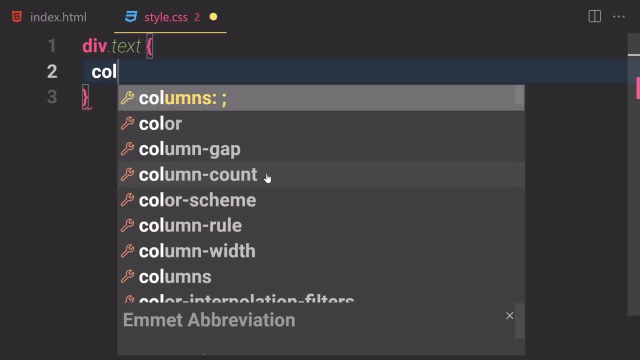 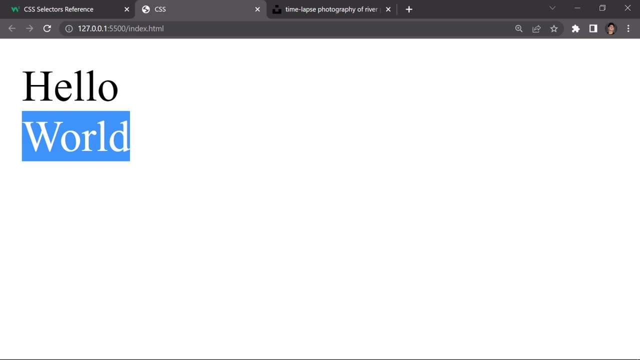 it's a text class, so now we can style that like: let's suppose if you want to change the color of it to like, uh, teal, just write a color of teal. and now, if you save that now, here you can see the style of the second div is changed to teal colored. that's because we 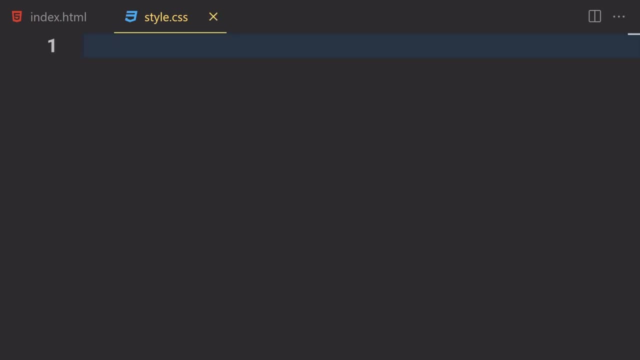 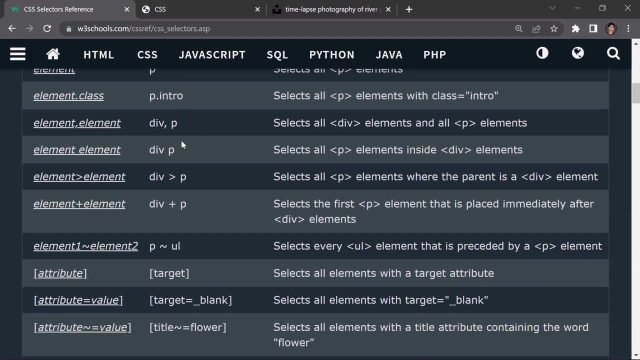 provide dot text uh clusters. so now, if you just remove that- and now we are going to be also removing these divs from here and i'm not going to be going through all of these selectors- you'll found that by yourself. but you know what? i'm going to just show you this uh div and p tag. so 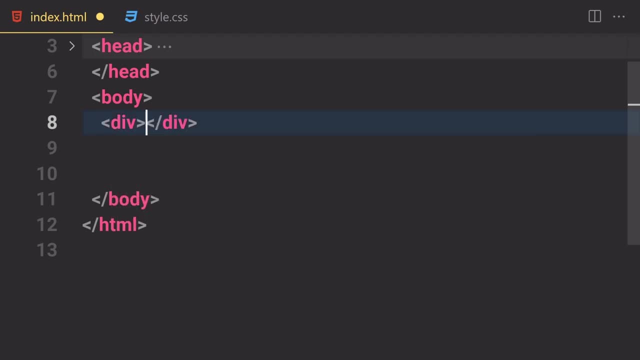 now let me just show you that real quick. and here i'm going to write div and then paragraph of hello, like hello, and then outside from this div, i'm going to create a new paragraph of word right here. okay, just a very basic examples i want to give you. so, first of all, we have a div. 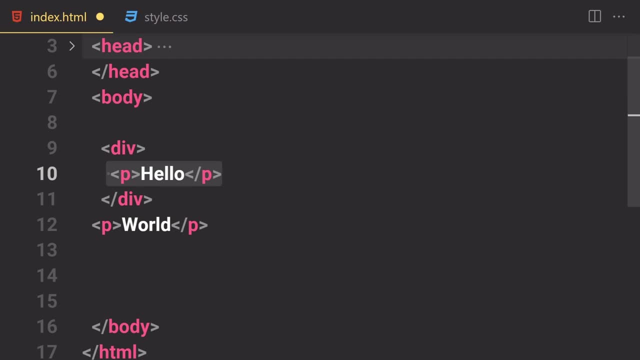 then we inside this div we have a paragraph of hello and then outside from this div we have just a paragraph of word. so now, if you save that and if you go toward css, so what do we have to do? we have to just write div and then p, and inside there we are going to be just writing a color of crimson. 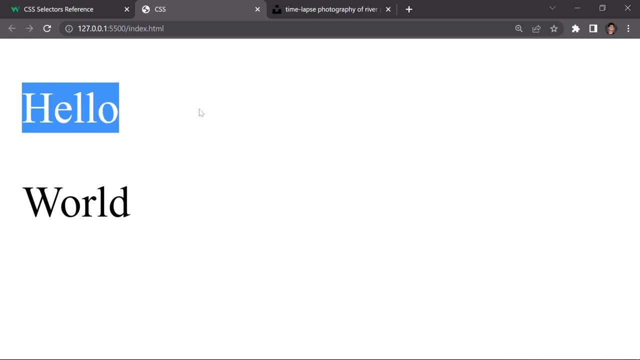 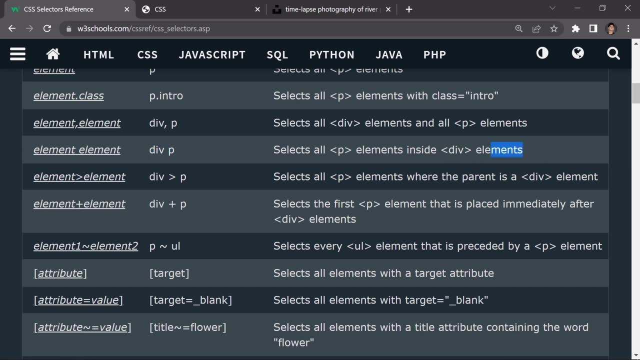 so here you can see it will now select this h1, the first hello. that's because it's saying in a definition like: select all of the paragraph elements of the div, and then we are going to write a div element inside a div element. okay, so it will just select every paragraph tag which is: 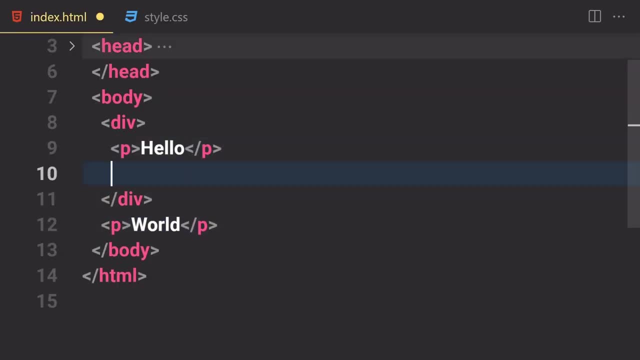 inside: uh, this div element right here. okay, so now let me just write h2 maybe, and i'm going to write like: uh, you know what, this will be. two. then i'm going to write: um, it's four of three. and then i'm going to write another paragraph tag and i'm going to write like four in here. and now, if you save, 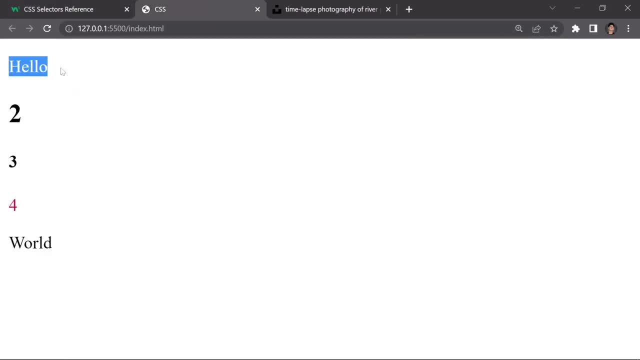 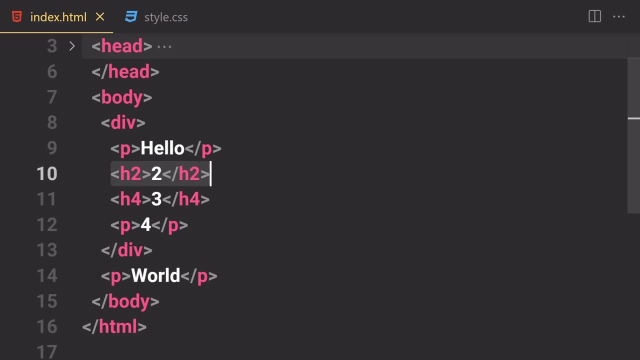 that and if we check, so if i just zoom out a bit. so now here you can see, this one color is changed and this one colors also change, and these two doesn't affect it. so i'm going to go ahead and check this one colors. all to be fine, i'm going to use this here. so this page color it will affect. 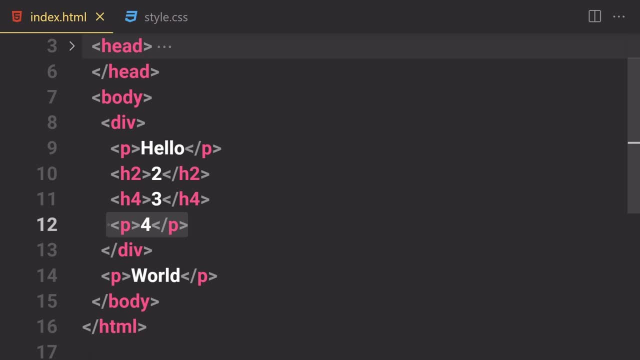 like, and if i just change the size square or the color, we will see if this is two equal or greater than 90. okay, now going to add another color. so like, if you make this a little bit wichtiger, this time also makes sense. right, let's make it a little bit more interesting. 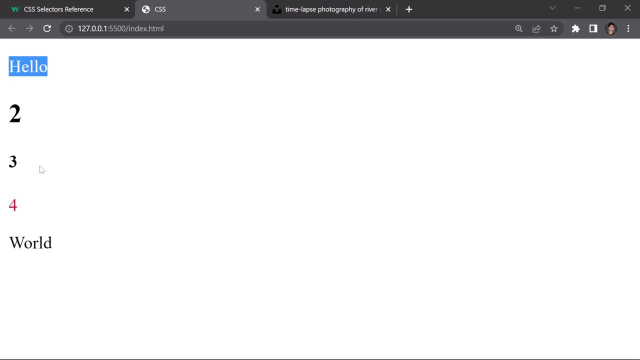 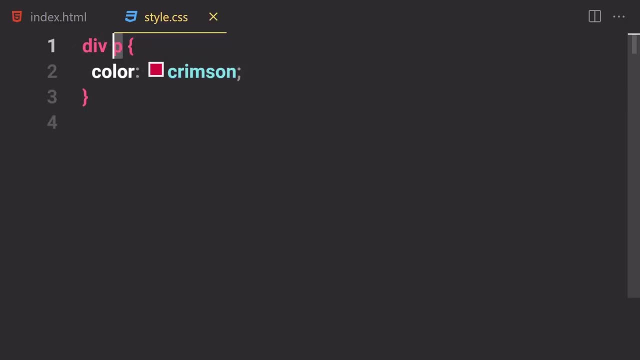 because if it was five points below than ten- and this one is equal to thirty five- we are going to have a div element and if that, instead of big, we are going to have Fragen, which we will default to eleven bars. so it's going to get smaller if we contract and key. 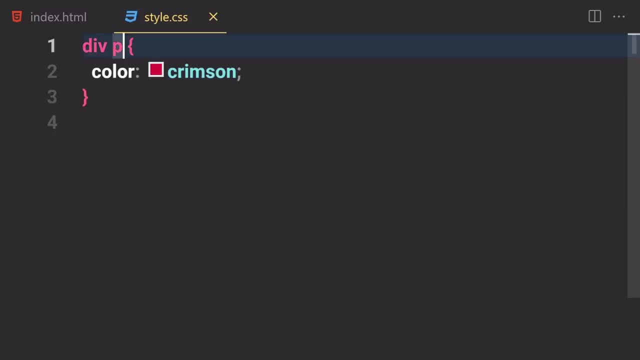 second is having this div element. it's going to become more longer than four if we contract this hold on a second. what we are meter and what we are going to do is we are connecting this two chairman pillar. so this is our theused, so that too, we have defined the previous sedan here. 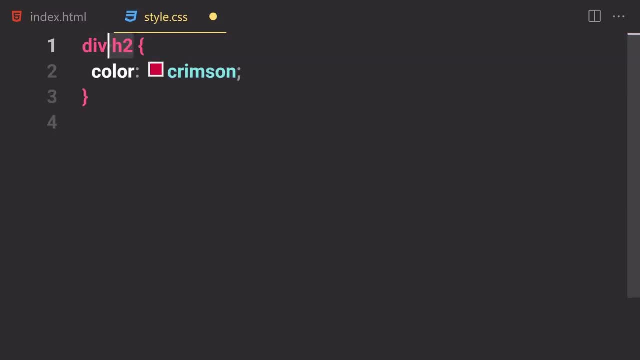 you can just write like div or any h2 which is inside this div, so you can now select. then, if you want to save our file, and now, here you can see this one, take your styling right here and the other one was ignored. so i'm going to remove all of this coding from here and also this coding from. 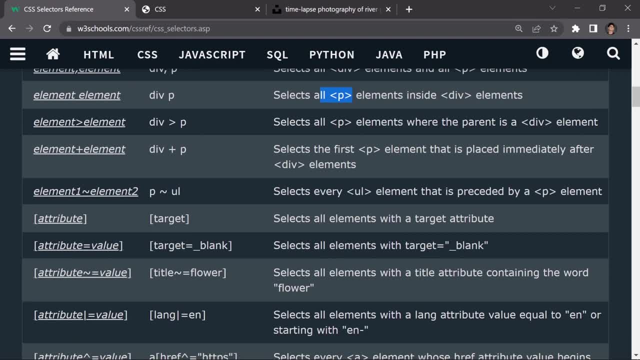 here as well. okay, so now the next selector which i want to show you is a div and div and grade and sign in paragraph. so what does that mean? it means, like, select all of the paragraph element where the parent is a div element. so it will now work a little bit different here. i'm going to just 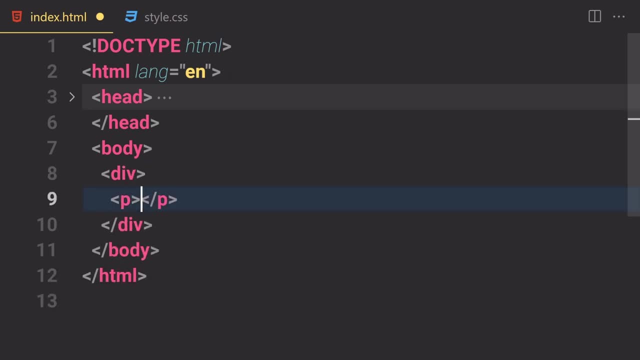 write like a div and inside this div i'm going to just write a paragraph. okay, so inside this paragraph i'm going to write hello, and then outside from this div i'm going to write a paragraph, and then here i'm going to just write a word inside there. and now, if you sell that, 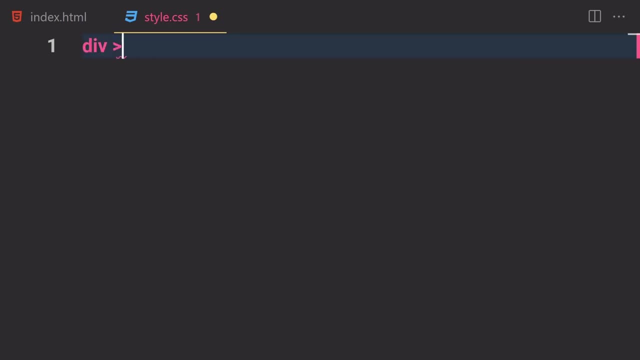 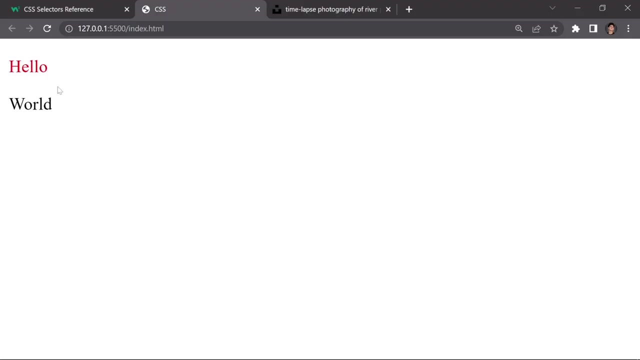 now i'm going to go to my css and now here i'm going to select my div and then greater than sign and then paragraph. okay, so here, if I want to change the color to be like red, so now if you save there and if you check it out, so 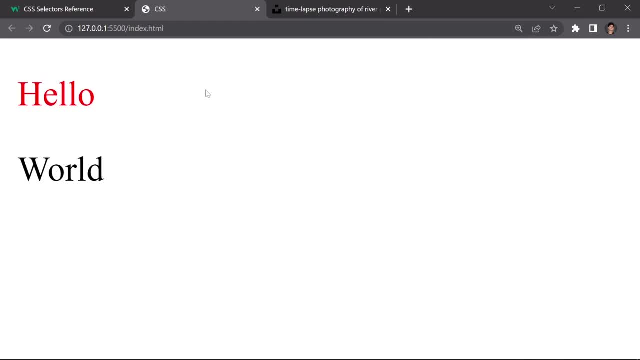 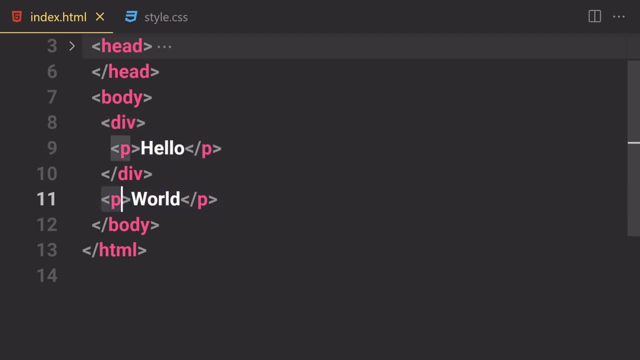 here. you can see this first one is affected. but if you just write something else, right here we have a div- then inside this div we have a paragraph with the text of hello and then outside from that we have a word right here. so now this paragraph is immediately inside this div tag. so this one. 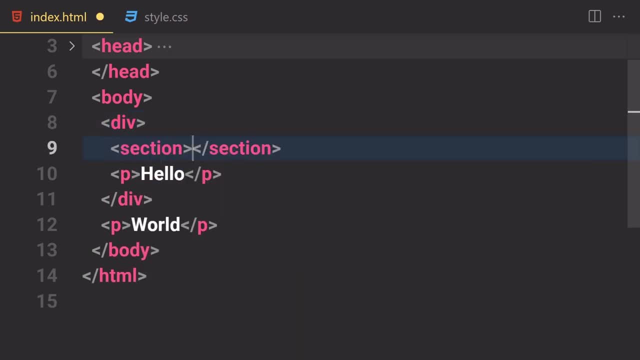 will take its styling. but if i just write a section in here, for some case, and if i just put my paragraph, if i cut it from here and if i put it inside this section, now guess what will happen? if you save our file and boom, that styling is gone, because this paragraph is not immediately. 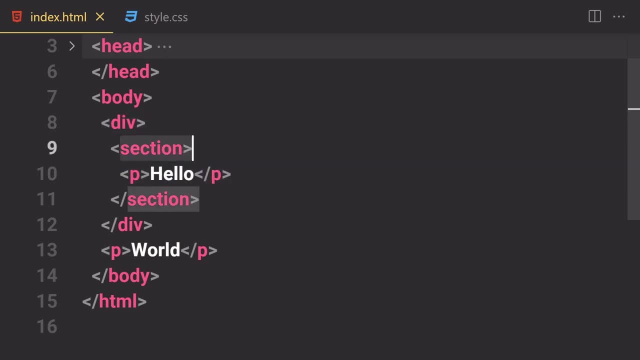 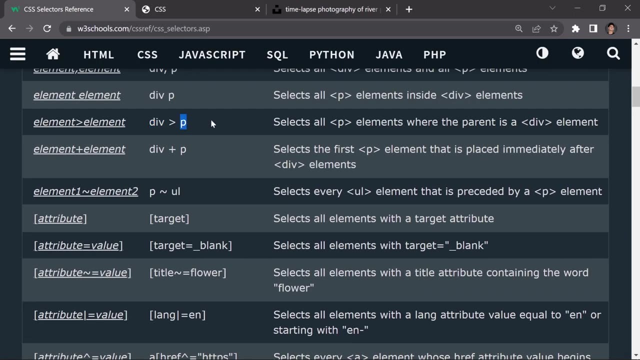 the children of this div. now, this is the children of this section, so this will not take its styling, okay. so now let me just show you that real quick, okay, so here you can see we have a div with a greater than sign and then paragraph. so select all of the paragraph element where the parent is a div. 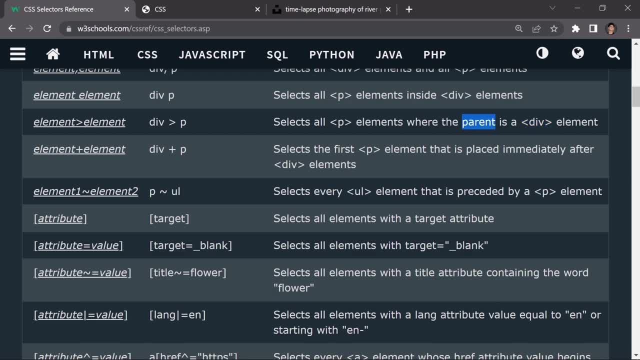 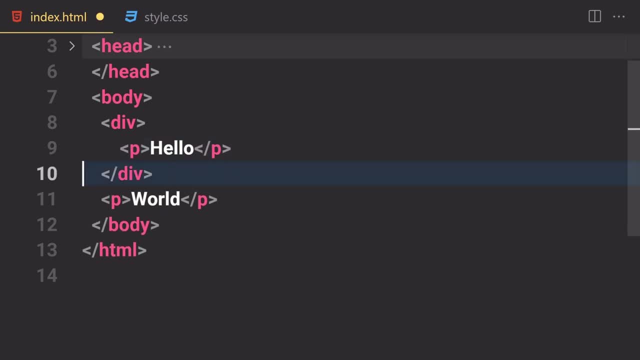 so the parent? i want you to notice this- the parent is a div. so now, in this case, the parent of this paragraph is a section, not a div. so if you just remove this section from there and now if you save our file, so it will take effect right here. that's because now the parent. 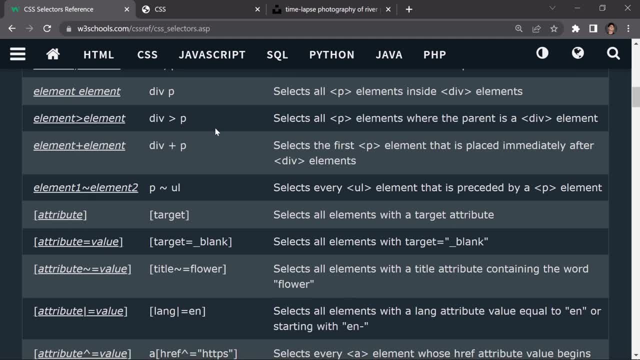 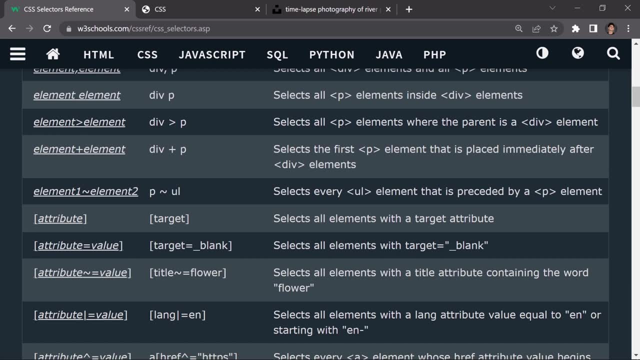 is a div. okay, so it will work like that. now, the next selector we have is a div and then plus paragraph, which means, like: select the first paragraph element that is placed immediately after a div element. okay, so what do we mean by all of that? now i'm going to go to my css and 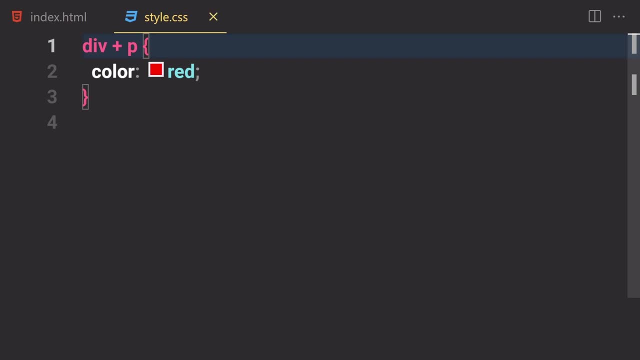 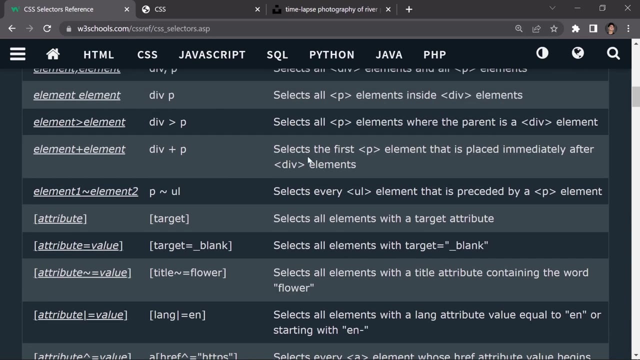 instead of this greater than sign, i'm going to just write a plus symbol right here and now. if you save that- and now, here you can see it will now select this second one. why now? in this case, they say like: let me just show you that: select all of the first paragraph element that is placed immediately. 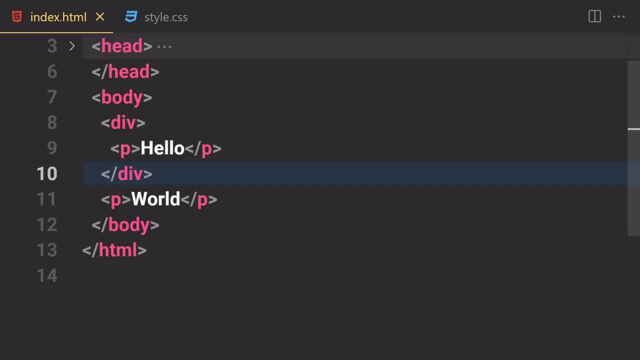 after: okay, so immediately after the div element. so what is immediately after the div element, immediately after? in this div element we have a paragraph. so if you just write like i don't know, maybe article in here, then if i cut my paragraph from there and if i put it inside this article. 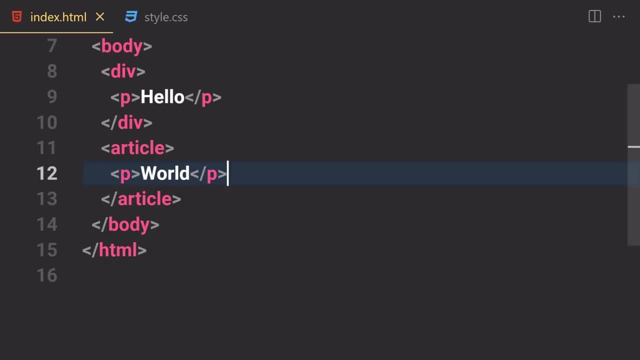 and if you save that and here you can see, nothing will affect it. why? because this paragraph is not immediately underneath this div right here. so if you just select all of the first paragraph element here, so that's why it will not be affected. okay, so now i'm going to remove that. and if you save 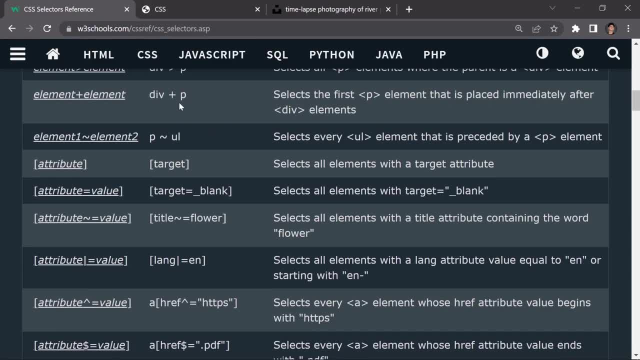 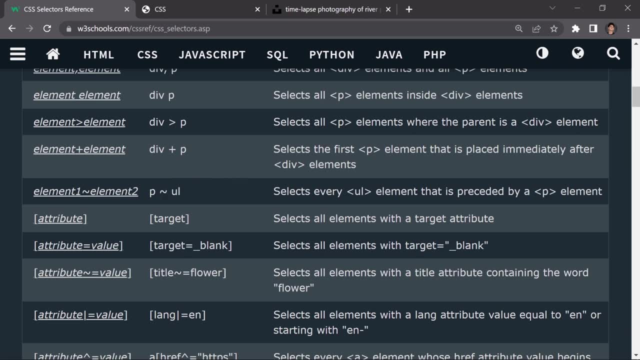 that, and here you can see this one is affected right here. okay, so that was quite simple and easy. and now the next one we have is a paragraph and then tilde ul. both of them are kind of the same, like um select every ul element that is preceded by a paragraph element. it is also like the same. 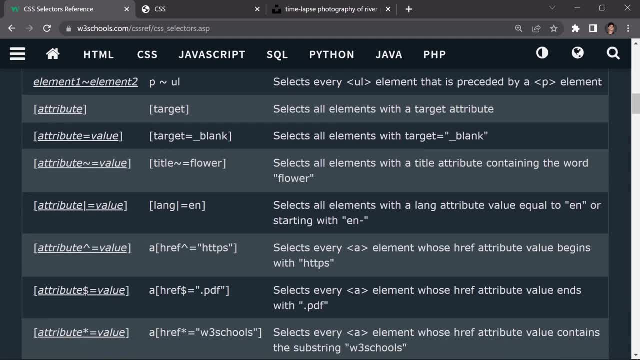 as this one. you can check that out, but i don't want to waste your time on that. the attribute selector: i don't want to get into like a specific attribute selector if you want to get more details, more about that, but in my opinion they will just waste your time. you don't have to like learn all. 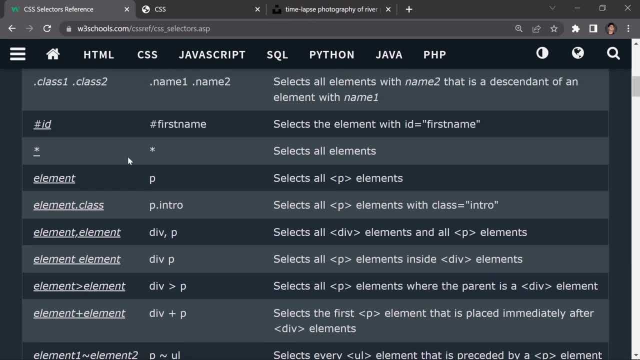 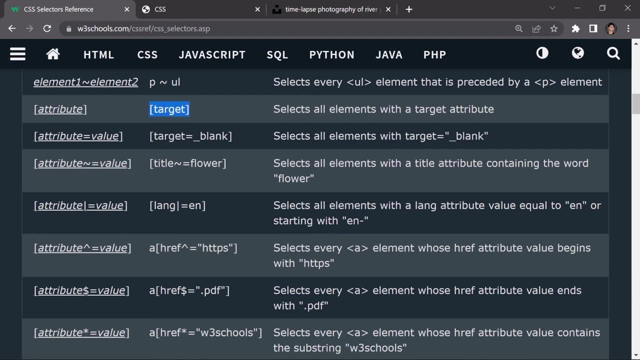 of them, but you will just use maybe a class selector or id selector. you will not use all of them, but you will just use some of them. so in this case, i just kind of want to show you this attribute one. so now, if you want to select something by attribute, so you just have to put 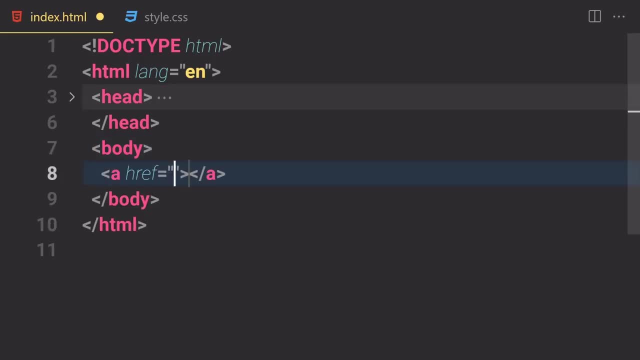 the inside this brackets. so now, if i want to write anchor tag with the attribute of this attribute, so i'm going to give him attribute of like. i don't know, suppose if i just give him an attribute of like one maybe, so a lowercase one, so i'm going to give him an attribute of one, and here i'm going to just 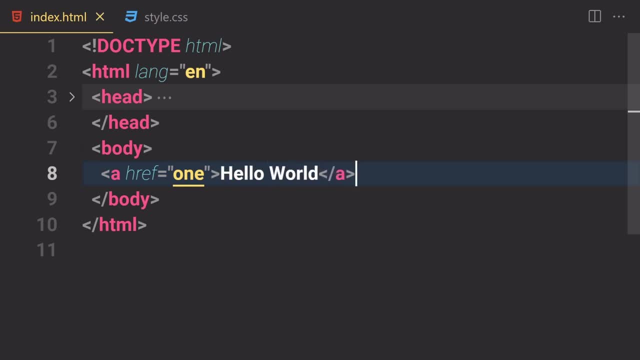 write like hello world. okay, so hello world inside there. now, if you save that, and what do we get? we get this like hello world right here and we give him an attribute of like one attribute and then one. so now if you want to select this anchor tag by using an attribute, so what do we have to do? 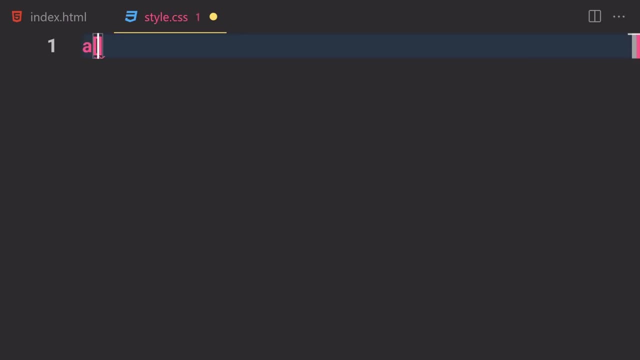 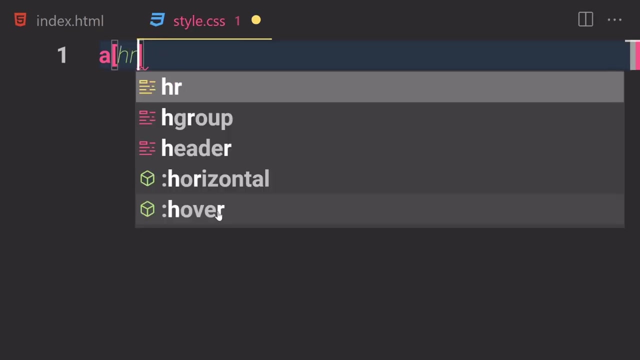 i'm going to remove this coding from here. first of all, i'm going to write an anchor tag and then i'm going to provide a specific attribute to it. so what is a specific attribute? i'm going to just write href h, r, e, f, and it will be now equals to one, okay? so if that's true, then i want you to provide a. 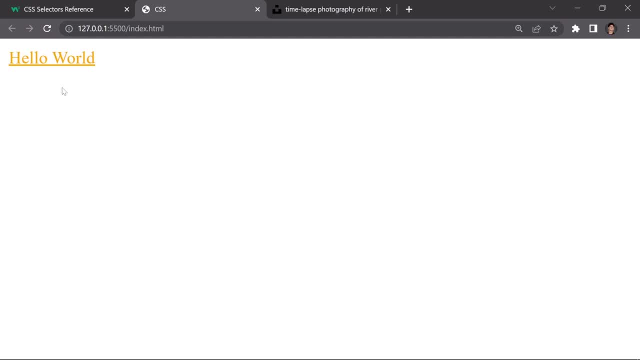 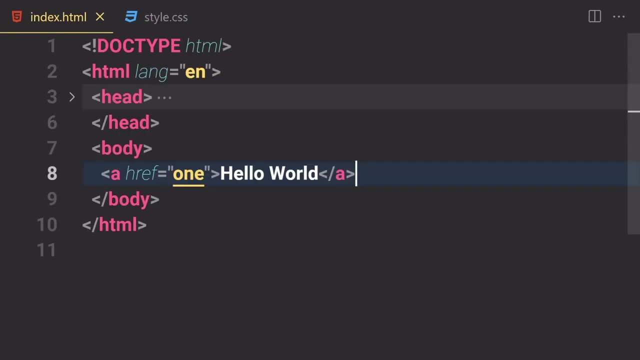 color of maybe orange. so now, if you save that, and here you can see, it will now provide a color of orange. so this is how we can select something: by using an attribute of href or whatever like. suppose if you have image with these two attribute and you want to select that by specific alternative. 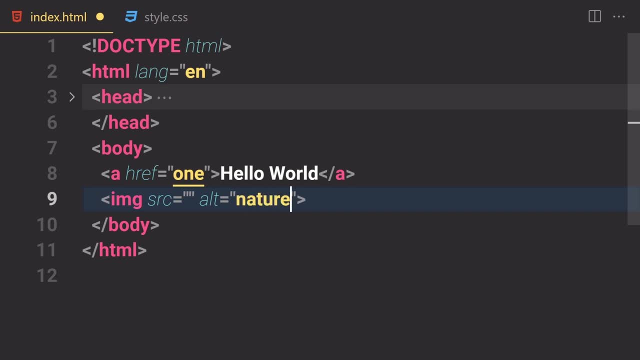 attribute like i don't know- nature or whatnot. so you can also select that by using first of all the img and then provide alt in here and then provide their nature or whatever you have, and then you can change the color of that and stuff like that. okay, so now i'm gonna remove that and 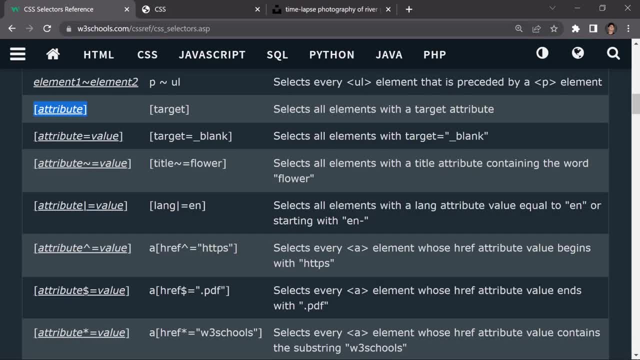 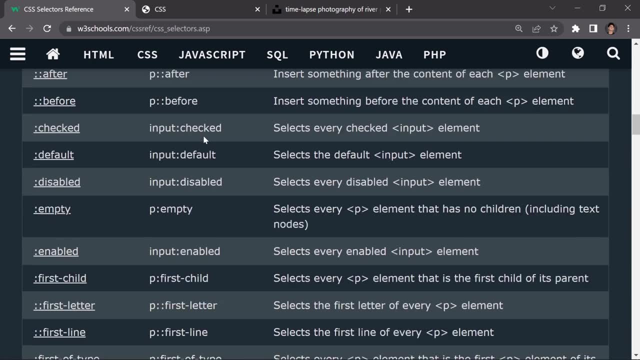 i'm gonna save my file and i'm gonna also remove both of them. save my file, the next one we have. you don't have to worry about all of these specific ones, okay? so i guess we are pretty much done with the selectors, okay, so the next thing which you have to learn is a pseudo selector. 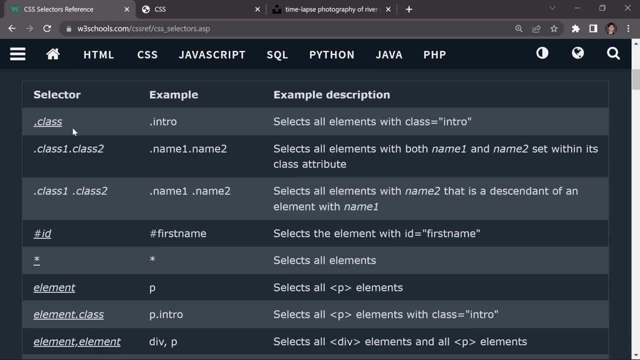 so now let's just learn about that. and, by the way, if you are confused about these classes and these ids and this specific kind of selector, trust me you are not going to be using all of these selectors in your project. you will either use classes or ids, and in some cases, you just use 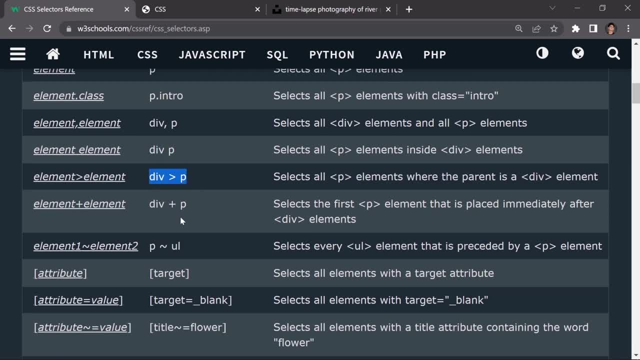 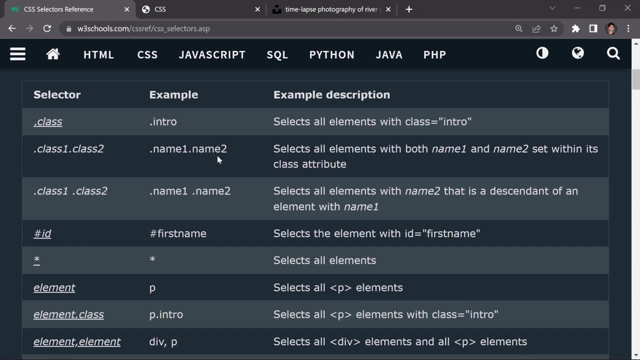 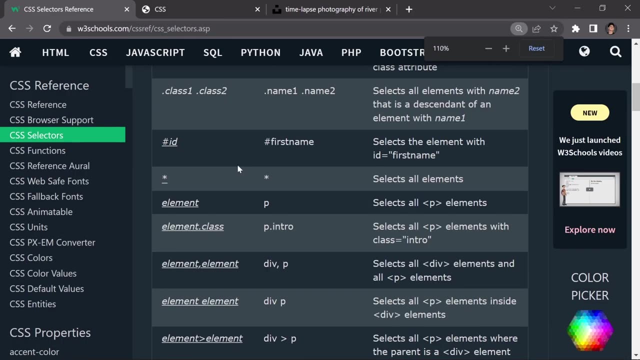 stuff like maybe these or maybe these, but not that much specific stuff like target selector or stuff like that. trust me on that, okay. so now let's jump into something called a pseudo selector. so now let's just look, learn about a pseudo selector. so we have a few pseudo selector like active, and active allows us. 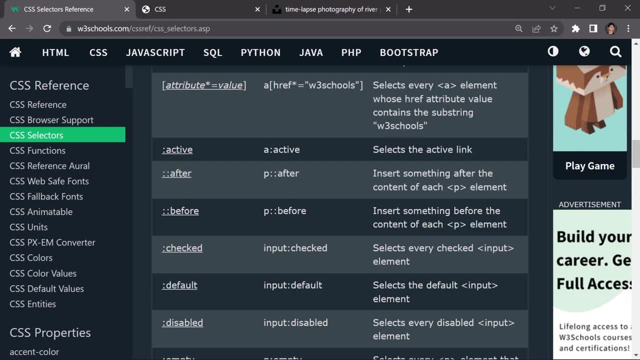 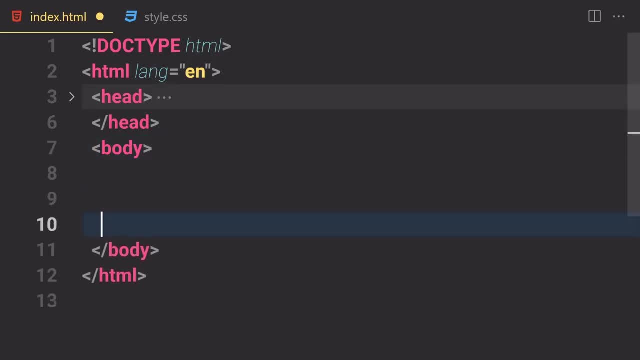 to like uh, select the active link. and these are four links, by the way, or not just only four links, but some of them are for links. so now let's just learn that, then you'll get to know what i'm talking about. so, first of all, we are going to be writing our anchor tag and then here i'm going to just 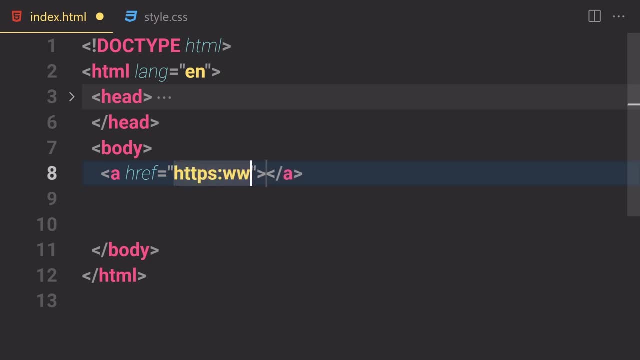 provide the link of like https, and then www, dot, um, some nyc- oh you know, i forgot to include this dot slash, slash. and then wwwnycgocom, which is like a new york tom website, and now i'm going to duplicate there a few times. okay, so now i'm going to change that to wikipedia, and now this one will be just a. 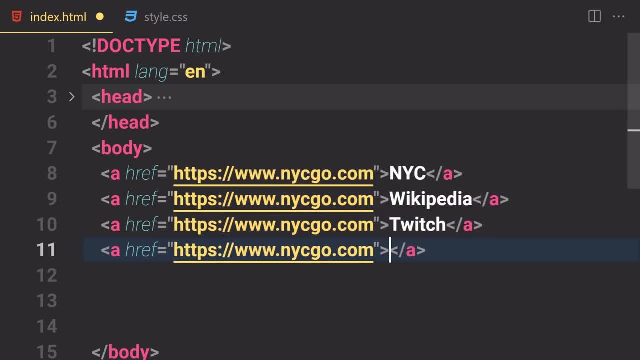 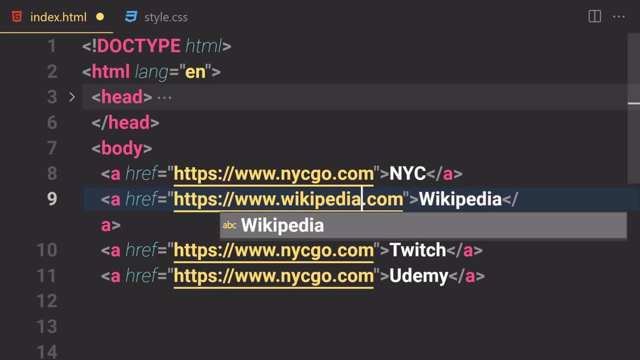 twitch, dot tv. and now let's just duplicate that. and here i'm going to just write like a udemy. and here let's just remove that nyc from there. and then wikipediacom. now the next one we have is twitchtv instead of dot com. okay, and now this one will be udemycom. so i'm going to just zoom. 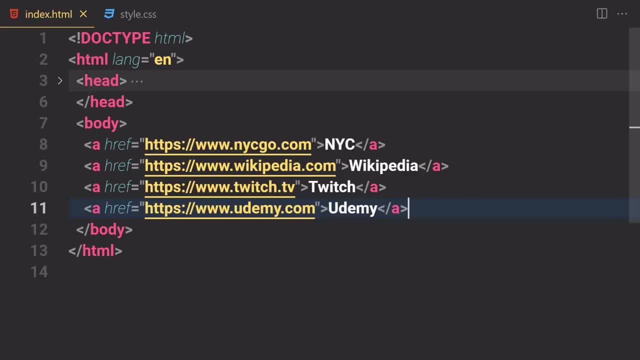 out a bit so you guys can see everything a bit clear. so we have just these links like uh, first of all we have a new york times, then we have wikipedia, then we have a twitchtv and udemy. so now i'm going to provide a specific classes to them. so i'm going to write a classes. 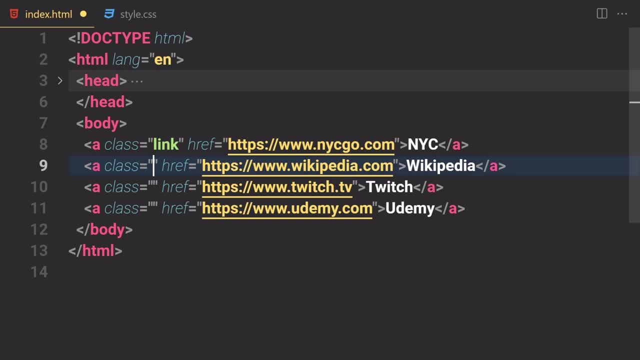 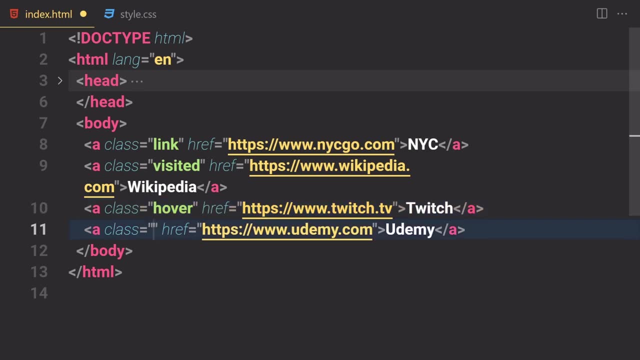 and hit tab, and here i'm going to just provide like a link class and then we have a visited class and also i'm going to give them a class of hover. this is my favorite one and we have an active one, okay, so now, if we save that now let's just start working on our links. so 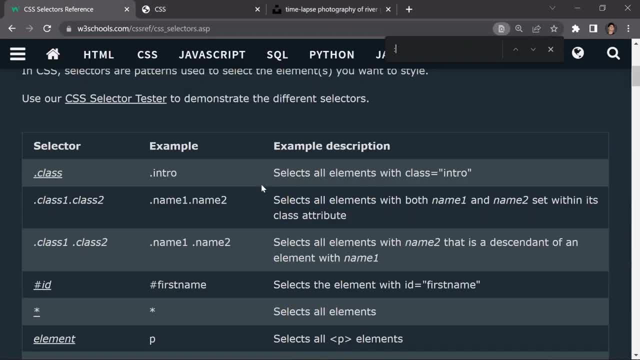 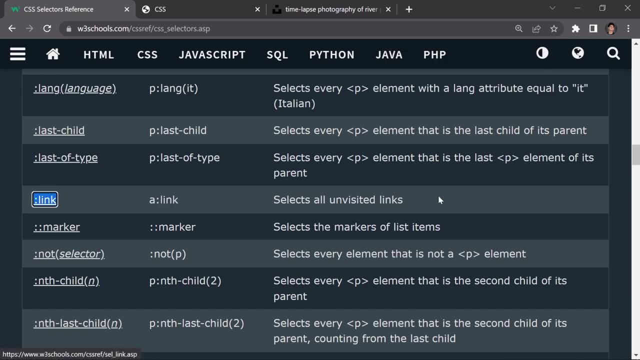 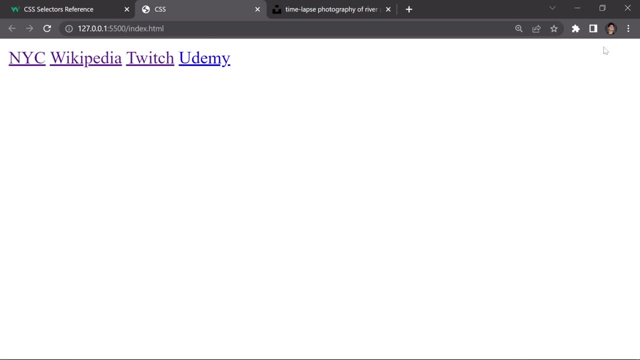 what is a link? first of all, let's just learn about that. so we have a link, so link is a pseudo selector. so select all of the unvisited links. so it will select all of the unvisited links. okay, so now we visited to all of these links, so what do we have to do? i want you to just click on these. 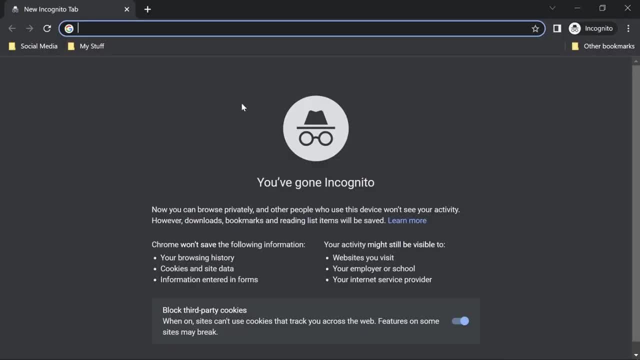 three dots and then click on this new incognito window and this is super awesome window. okay, you can see how full stage this window is, that it doesn't have any history tabs right here. okay, so you don't have any history tab. you can just like search anonymously inside this incognito. 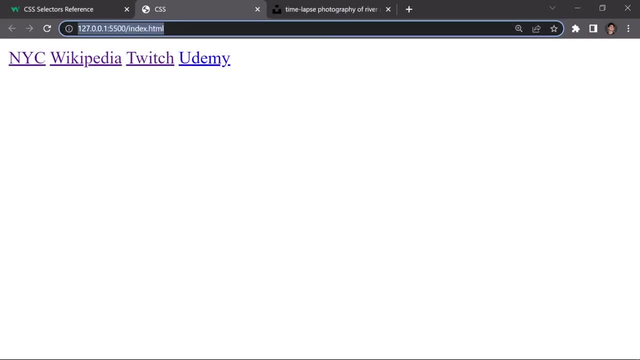 window if you want to, okay. so what i'm going to do is that i'll just copy this url and i'm going to paste it inside this incognito window, and here you can see, it will now gives us all of the links in which we didn't visit. so now let's jump in towards css. and now here you can. 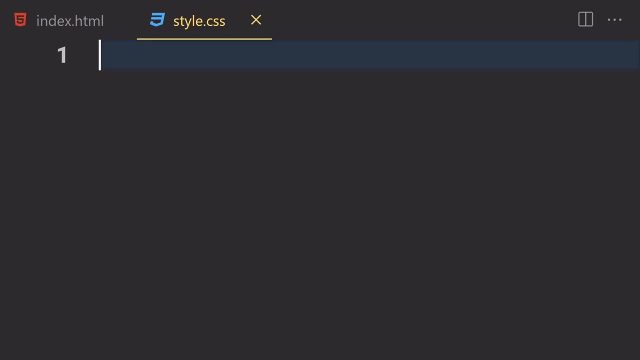 see, we have this link. so now, if you want to select, that first of all we provide a class to it, so we'll we have to do, we have to write a period or dot, and then we have to write a link- not a link but a class name- and then, if you want to select a pseudo selector, so for that we can just either: 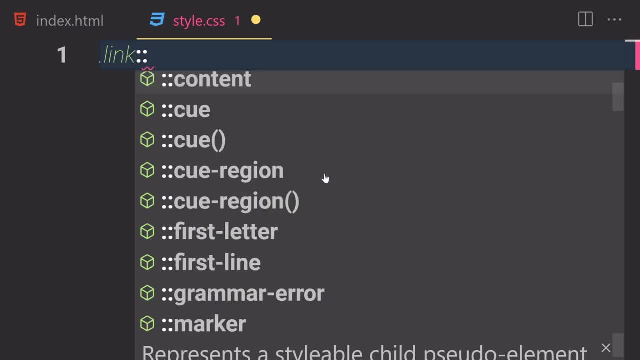 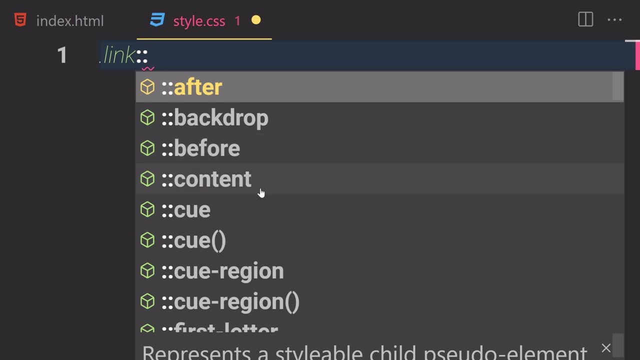 use one colon or double colon, it will give us all of the list of pseudo selector we have inside our css. you don't have to worry about all of them, because we are going to be learning about the majority of them, like those which you would need. okay, so here i'm going to just write a link. 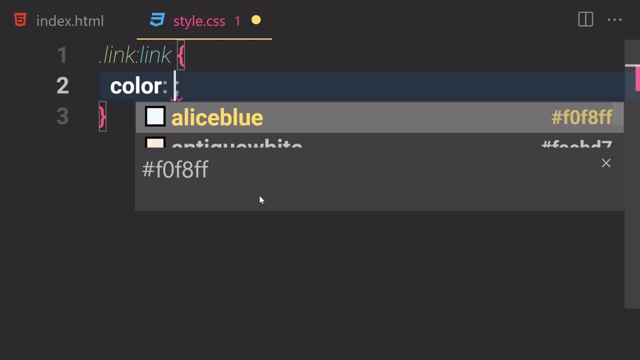 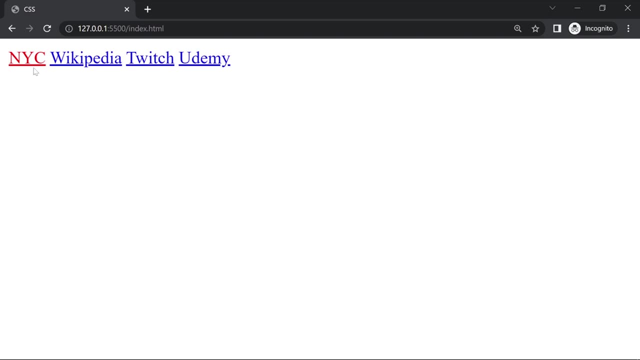 and now if i just select that and if i write like color of: maybe red, and now if you save that, so here you can see, it now gives us a red color right here. so we didn't visit to this link, so it will not use a red color. but if we visit to this link, like if i click on that and if i visit to this, 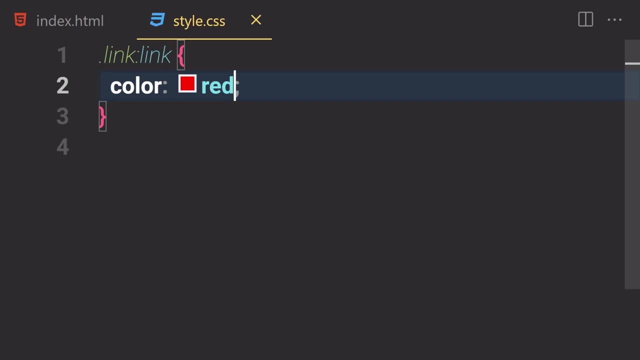 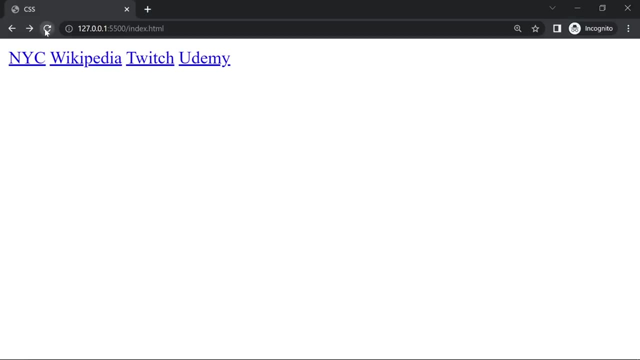 side and if i go back, so here you can see that color is gone. so this is how the link pseudo selector works. you can either provide a single colon or a double colon, okay, so if you just save that and if you okay, so i guess in this case double colon doesn't work, you have provided. 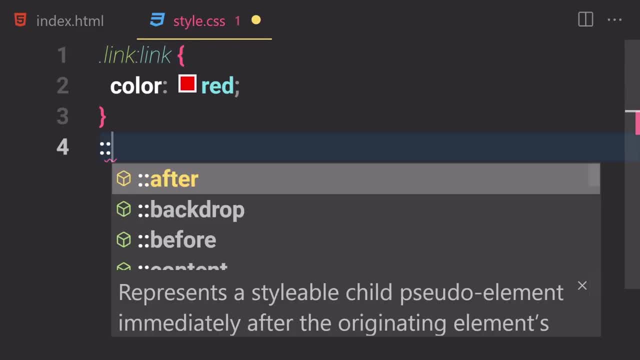 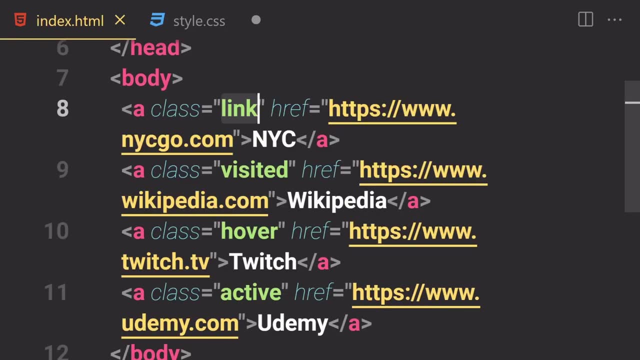 a single column, but if you want to work with a before and after selector, you have to provide, like, uh, double colons in there, and i'll highlight that once we get into there. okay, so now the next thing i want to select is visited one. so now let's just learn about that. like what is a visitor? 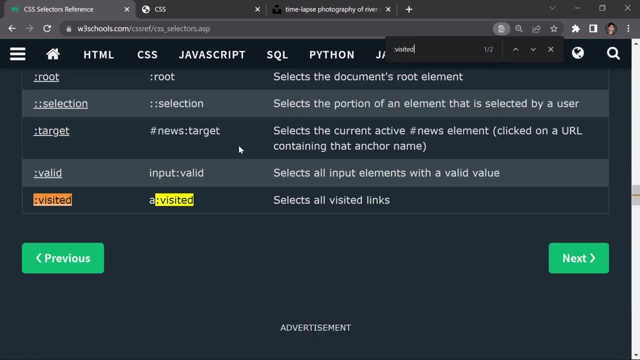 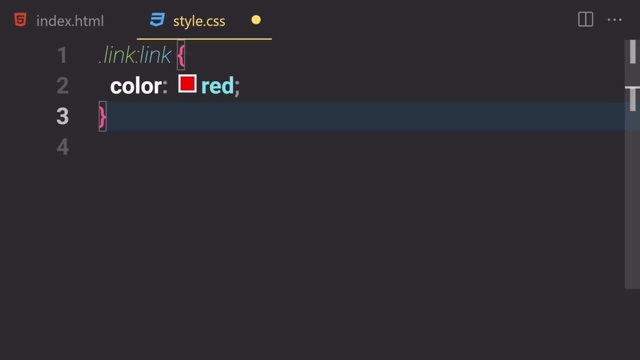 and then i will tell you v-i-s-i-t-a-d. so select all of the visited links, like those link in which we wizard. so it will now select all of their links, uh, which we visited. so now let me just select that visited and then let me just try to visit it in here, and i'm going to provide a color of blue, okay, or blue. 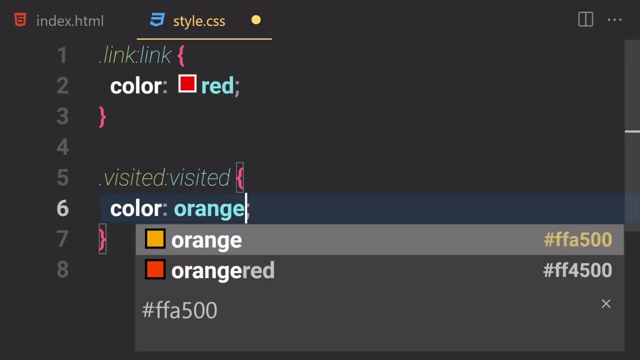 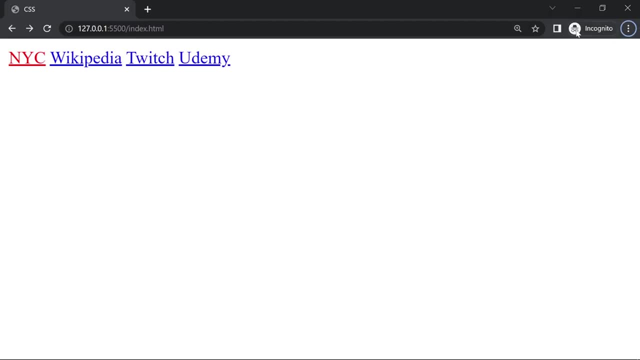 is by default, but you know what i'm going to provide: a color to be like orange maybe, and if you save that and if we go to our original- not incognito, incognito is this one. here you can see these uh kind of um glasses and stuff and this is our original. if you go there and now here you can, 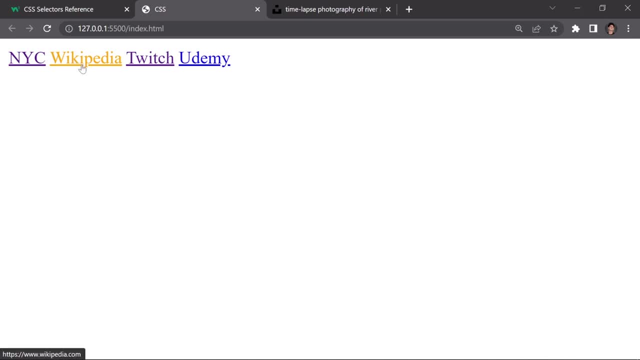 see. it will now select this one, because we already visited to this, uh, wikipedia. but if you click on that and go back and here you can see, that color will be gone. okay, so that was it about for a visited one. now the next one which you are going to be learning about is something called a hover. 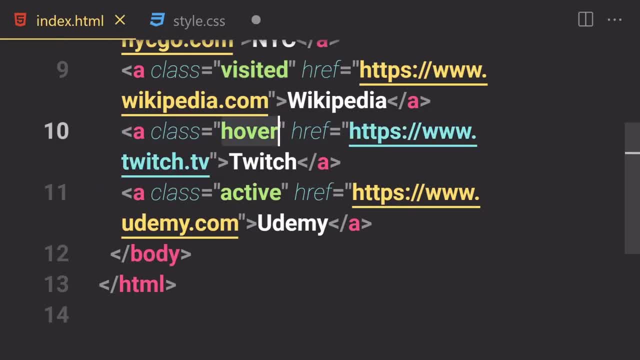 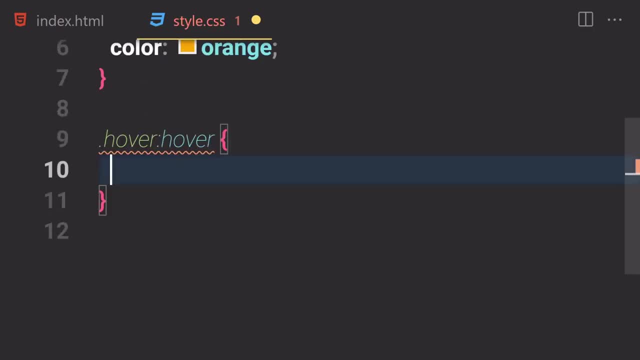 and how it is my favorite one. you can use that for anything you want, not just for only four links. so i'm going to select my hour and then let me just try to hover inside there. so here, what we have to do is that we can change the color to be like, maybe, um, sky blue. let me just write a sky blue. 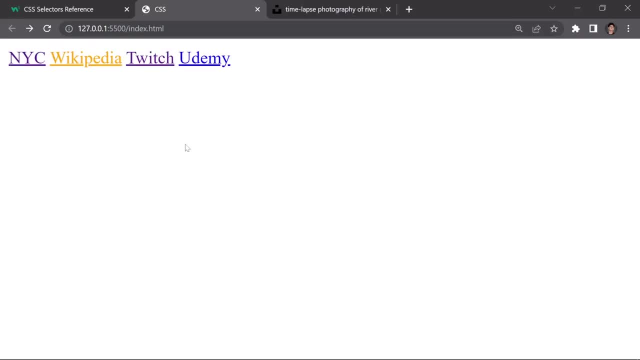 color. and now, if you save that, and now, if i hover my screen, i'll just select my hour and i will just mouse over to this uh twitchtv. so here you can see, it will now change the color, and if i just hover it back, it will now just remove that color if we hover over it again. so it will now just 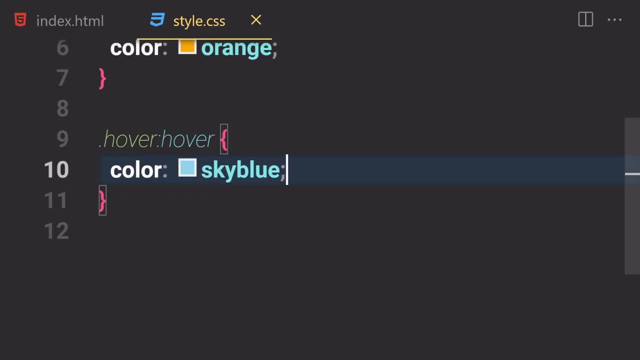 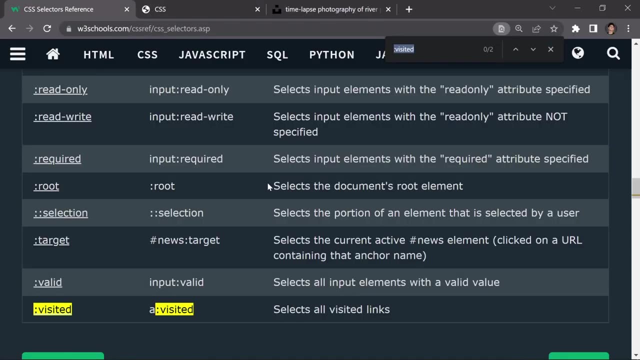 change that once we hover our mouse over to it. okay, it will change the color. now the next one we have is the active one. so we have this active one, but before we do, let me just show you the active one and select all of the active links, like those links in which we can click on and 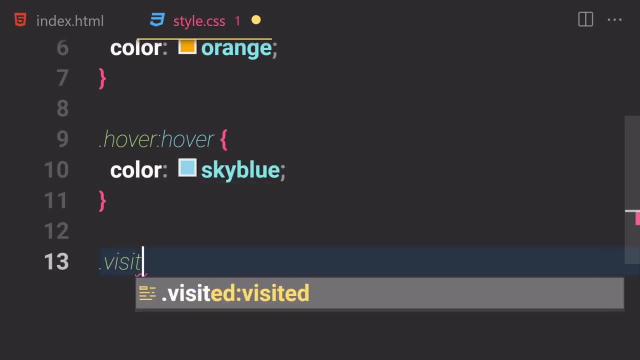 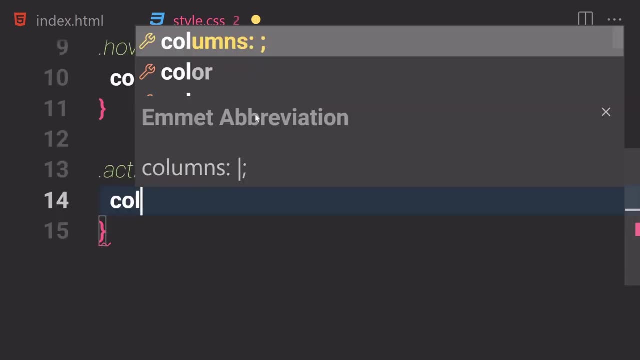 it will bring us to that page. so if i just select my wizard- uh, not wizard but active one- and here i'm going to just provide like active, uh, pseudo selector, and here i'm going to just change the color to be like i don't know which kind of color would be fine, i'm going to give him a teal color. 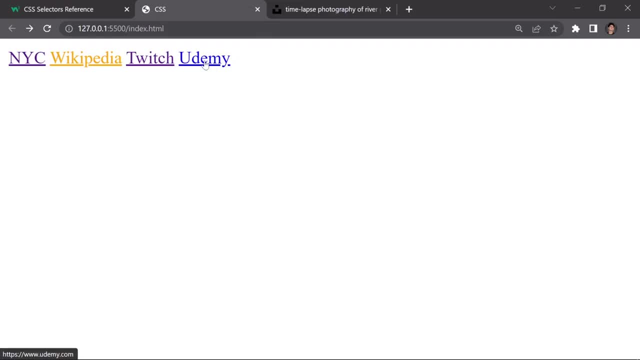 i just know these few colors. so now the final one we have is this: uh, udemy, and if i click on there- so here you can see- it will now change the color to tly because this is now active. so i am now holding my mouse if i just throw it somewhere. 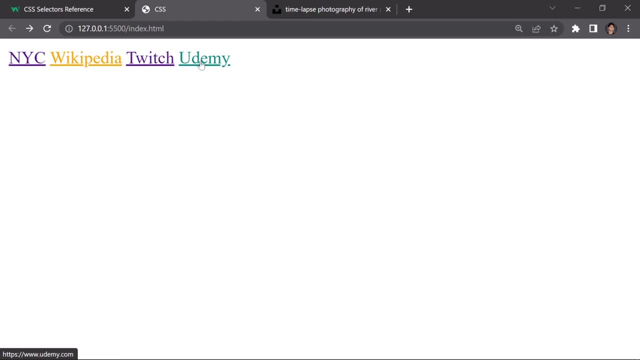 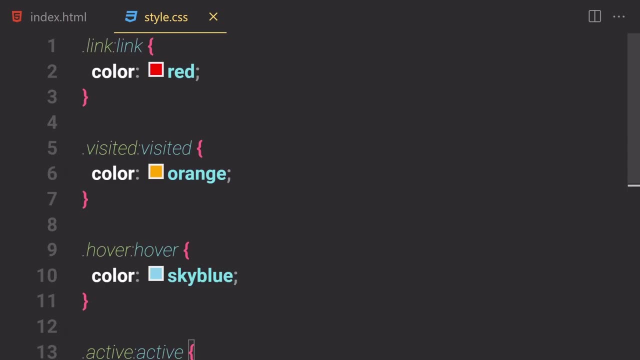 else it's blue. if you click on it one more time, so it will be teal color. okay, so these are a few pseudo selector which i want to show you in this section, but we are going to be learning about a more crazy pseudo selector later on in this section, so i'm going to now remove that, okay. 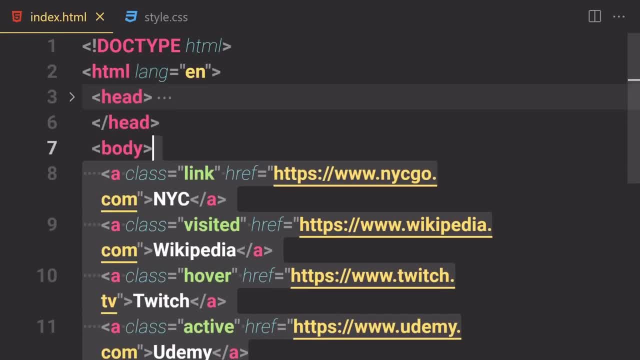 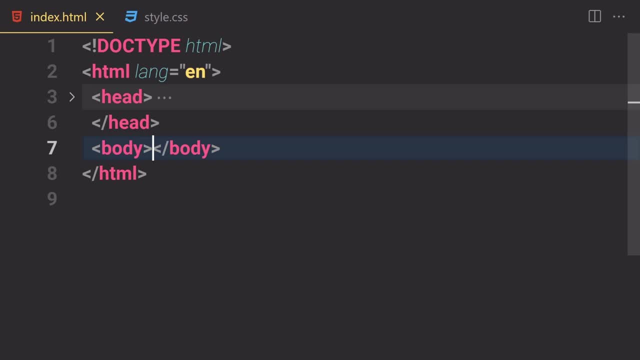 and i'm going to also remove all of this code right here now that we are done with selectors and a pseudo selector and stuff. so now it's time to learn about a display properties. okay, so so by default, if you write some html elements, so some of them will have a display of block and some 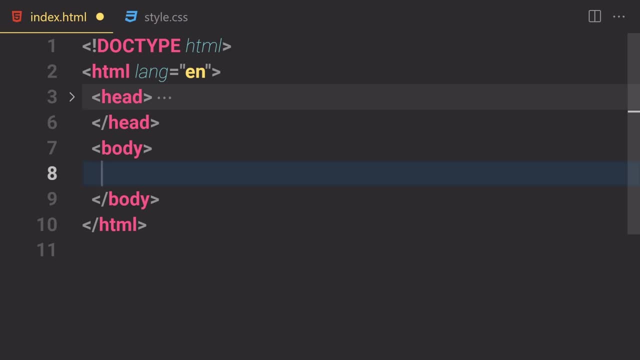 of them will have by default the display of inline. okay. so if i want to just write like uh div, so div will have a display of block. and then if i want to write a span, as i showed you in a previous video- and not a video, but in this section, in a previous section- and if you just write like uh inline, okay. 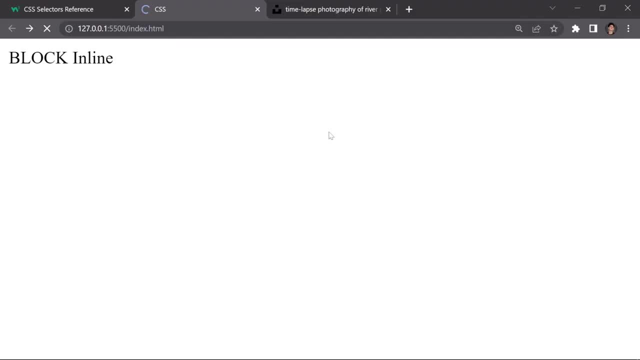 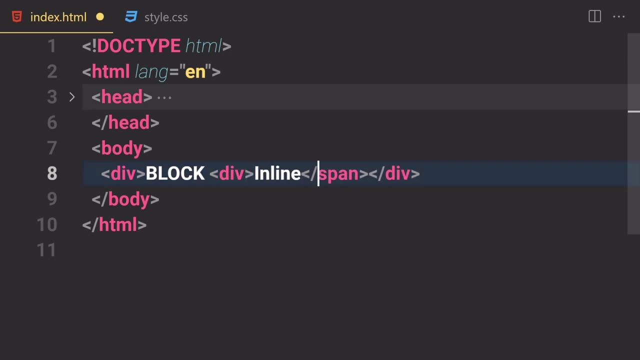 so i want you to just notice these two and if you save that and here you can see both of them are in right here. why is that? if i just change that to instead of from uh span, if i change that to like div, and if you save that and here you can see both of them are in new line, what's going on with that? 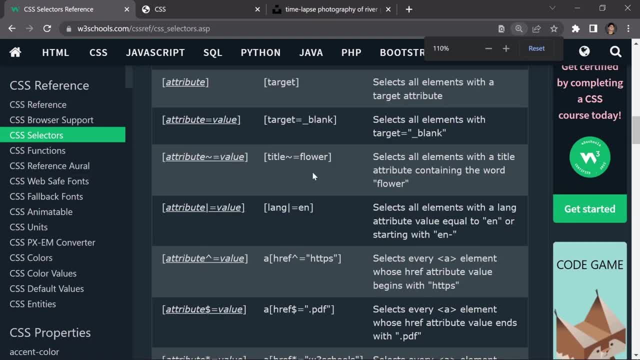 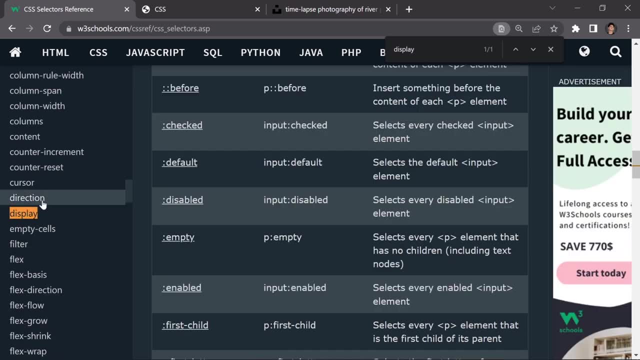 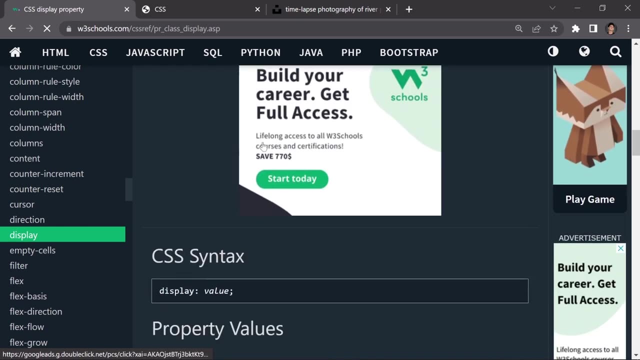 well, so for that we have to go to our w3 school and ask our girlfriend, like what's going on. uh, someone will just write like a display property d-i-s-p-l-a-y and i'm going to click on that. and now, here you can learn more about that. but i will recommend you to, not because i'm 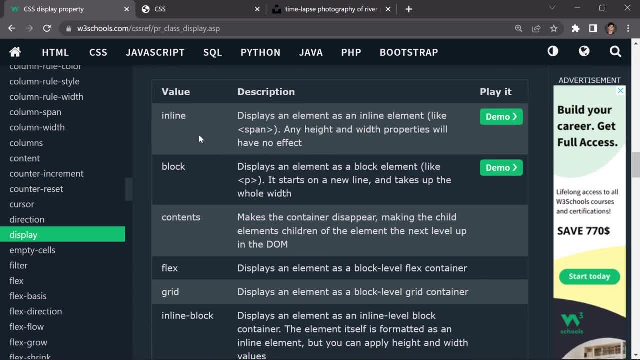 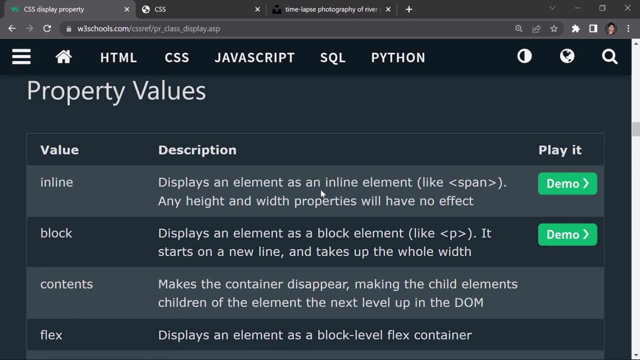 telling you, so why would you waste your time again and again? so, first of all, we have an inline property. so so, inline. first of all, let's learn about inline one. display an element as an inline element, like a span, which i showed you just a second ago. any height and width property will. 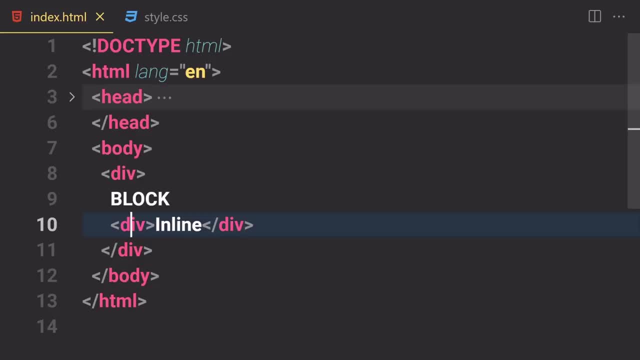 have no effect on there. so if i just write like: instead of uh, there, div, i just write like a span in here and if i write, spend one more time if you save that. and now if i want to select that and by using a span tag. so if i just write like: 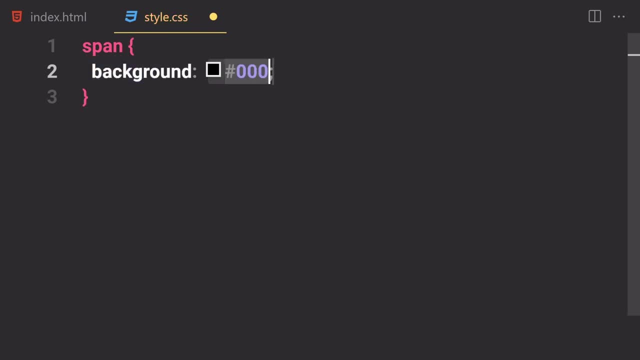 span. and now, if i want to provide, first of all, let me just give my background color to be like, uh, maybe teal, would be fine. so if you save that and here you can see, now we provide this uh, teal color to it. and now, if you want to provide the width or a height to it, so it will not take. 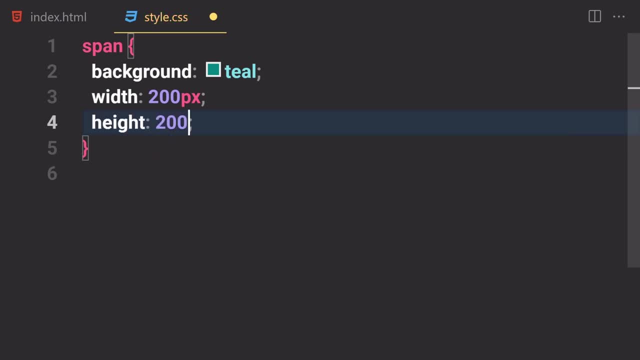 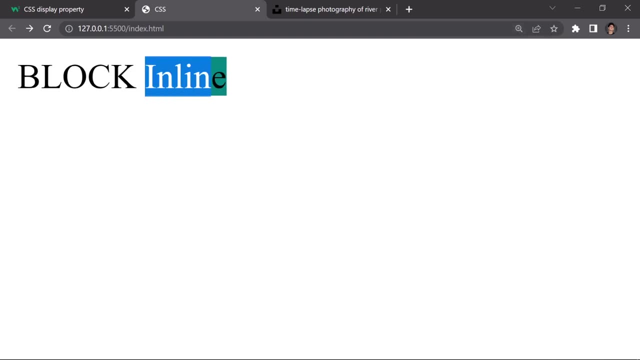 that if i want to provide a width of like 200 pixel or height of 200 pixel, and now if you save that and boom, nothing's going to happen right now because we are totally working on just an inline uh display, so that's why it's not taking a width and a height as well, okay, so on. 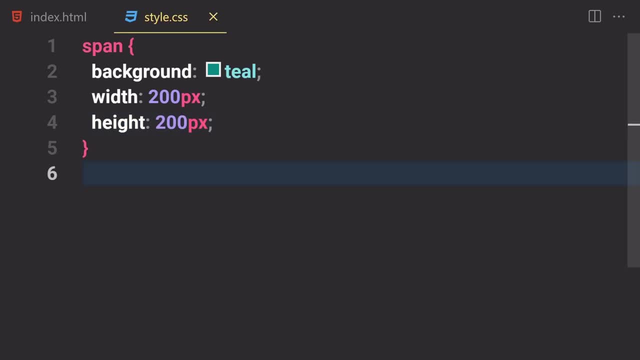 the other hand, if i want to select my different here, if i try to provide these width and height to a div instead, if i want to select my div right here, like this one. so if i want to just write div, and now let me just copy all of the code and i'm going to paste it right here. 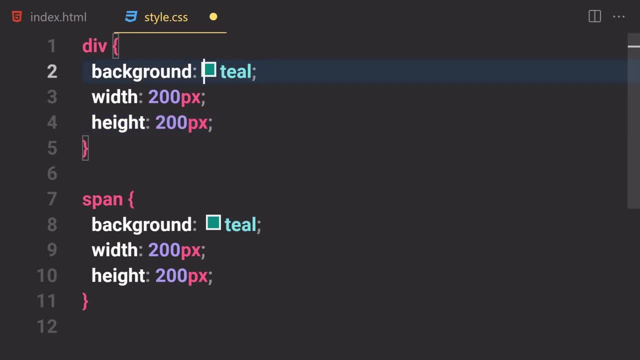 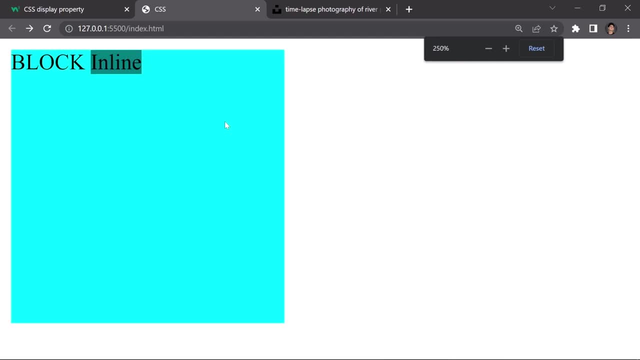 but i'm going to change the color to be like, i don't know, maybe come on, cyan would be fine. if we save that and here you can see, it will now take this width and or height one as well. so if you just change that to 100 by 100 and if you save that, so here you can. 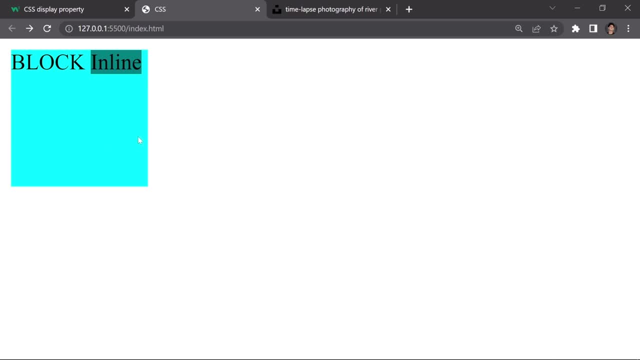 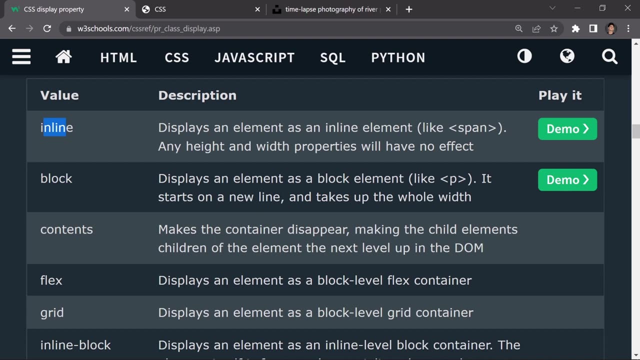 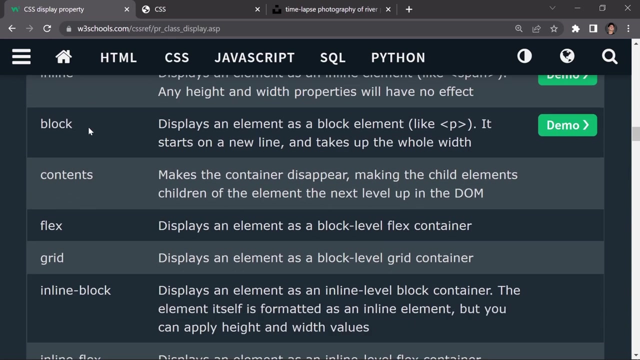 it will now take this with like 100 by 100, like 100 of width and 100 of height. so what is going on? okay, so this is an inline one and, as we learned that inline will not take a height and, with property, the width and height property will no effect on an inline element. on the other hand, we 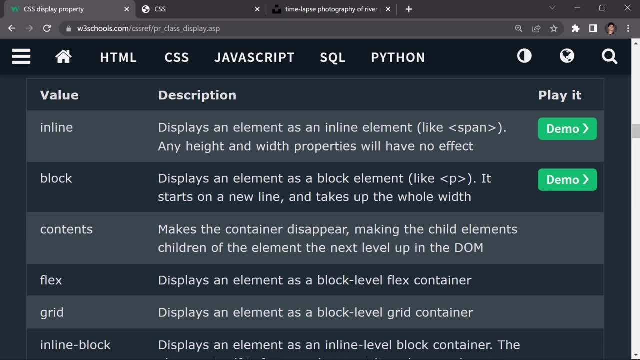 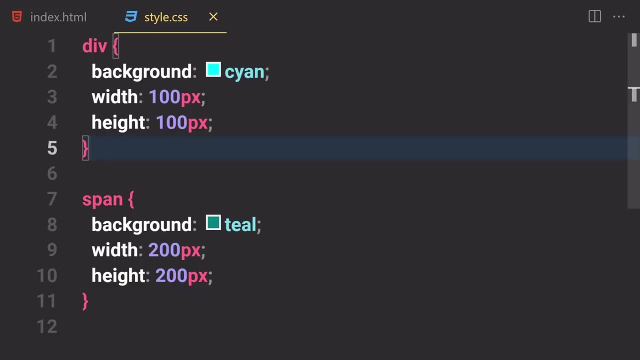 have a block one, and block displays an element as a block element, like a paragraph or div or section or a header or footer or article main and all of these semantics which we learned in a previous. it start on a new line and it takes up the whole width. okay, so, uh, any block level element will. 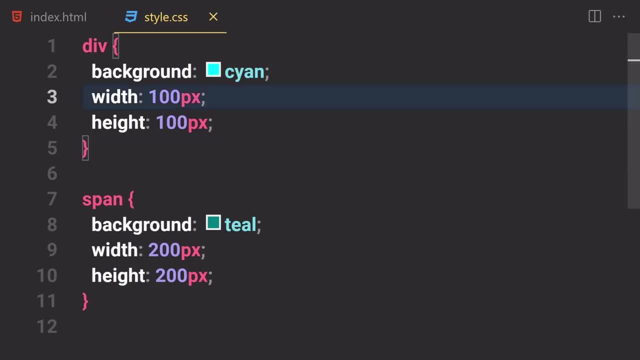 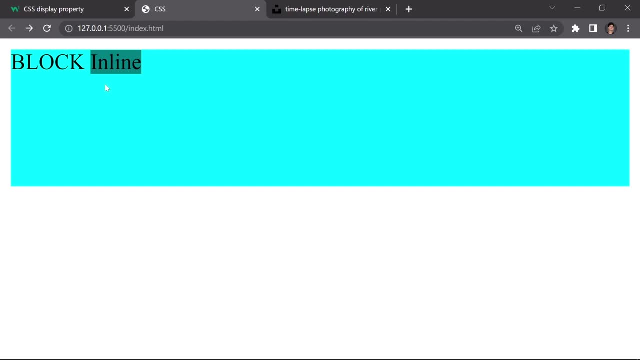 take all of the its entire width. so if i just remove this with from there and if you save that, so here you can see, it will now take entire width and anything come up in the front of it, it will just remove that and take entire width of it. okay, so on the other hand, we have um inline one. 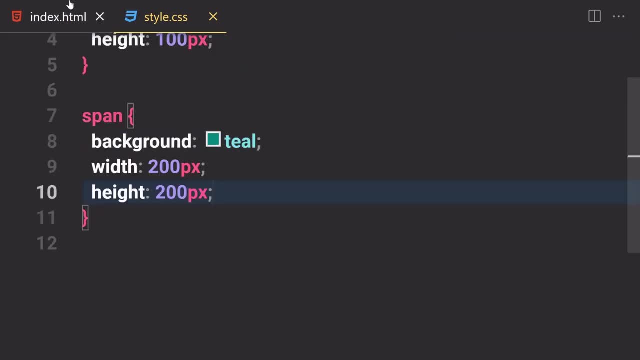 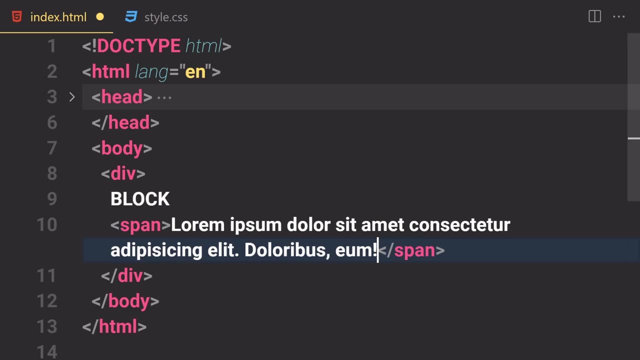 inline will not take its entire space, but it will just uh work on its content, like if i just write a lot of content, uh, and draw some rock on it, uh, and then i'll remove it. so also you can do that here: uh like lorem maybe, uh, lorem 10 maybe, and if i hit tab and if you save there and here you can. 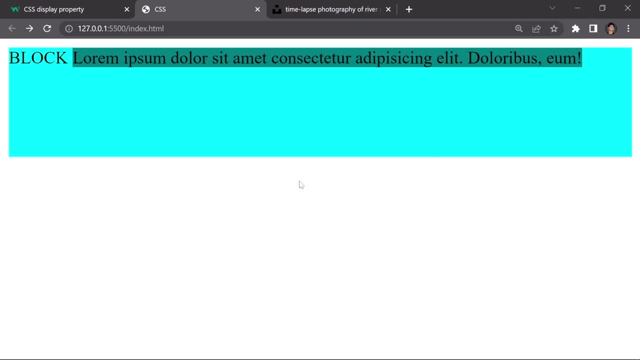 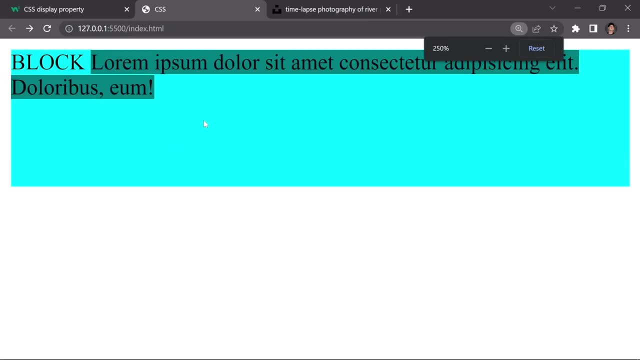 see, it will just take its content place, but it will not take the entire width. okay, so this is the difference between the display inline and display block. okay, so now, in some situation, we would need to provide display of inline, but we would also want to provide uh, width and height. 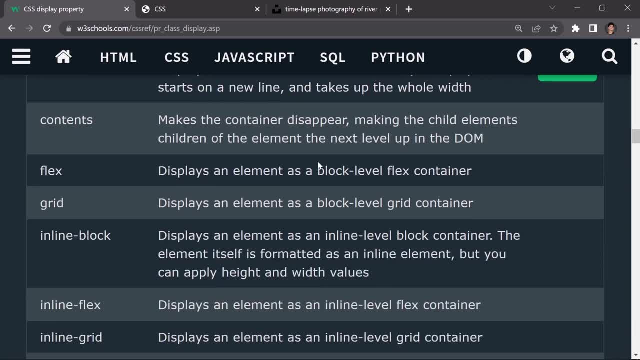 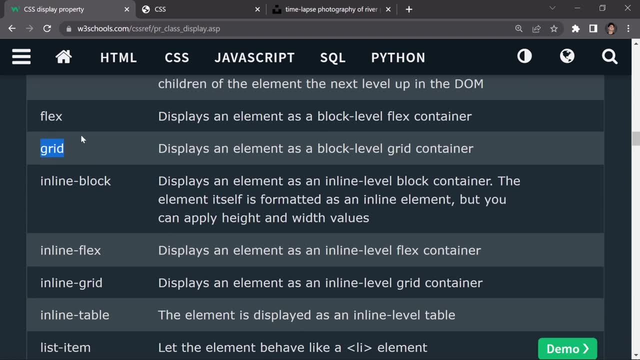 to it. so for that, we have another special property called inline block, and you don't have to worry about um flex and grid- these two are my favorite one, but you don't have to worry about them for now- which we are going to be learning in a really, really great detail later on in this video. so now, 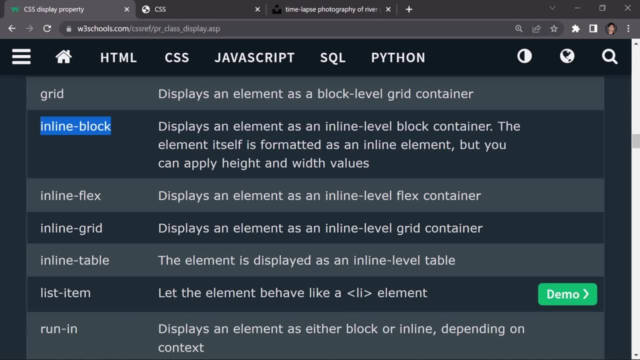 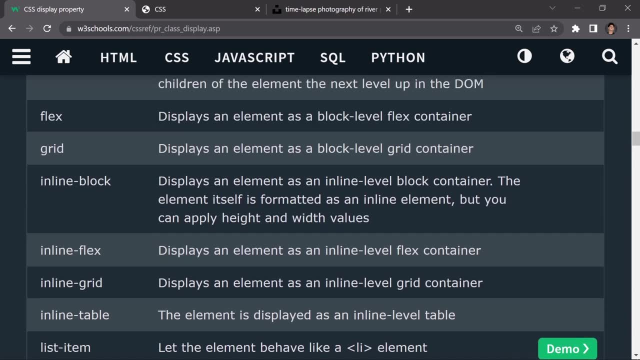 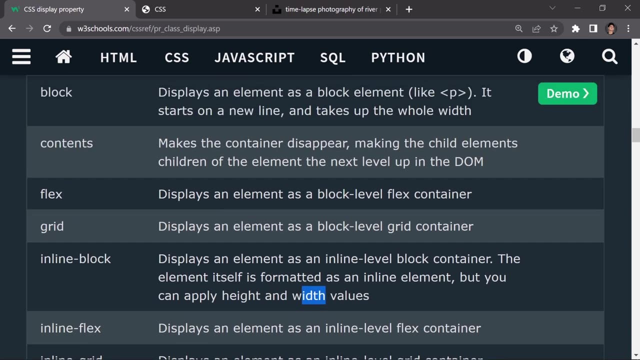 we have inline block, so inline block displays an element as an inline level block container, as we learned that in here, just in inline one. but in this case, like inline block one, the element itself is formatted as inline element, but you can also apply hide and with to it in just an inline we. 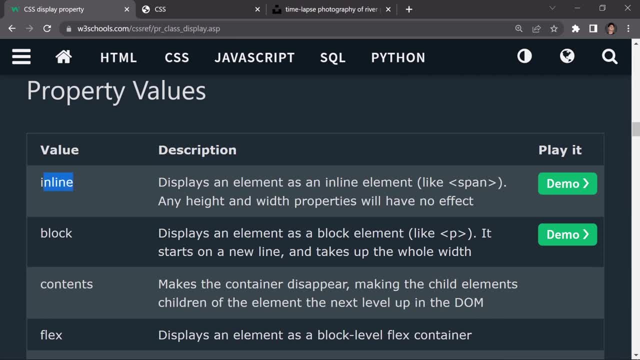 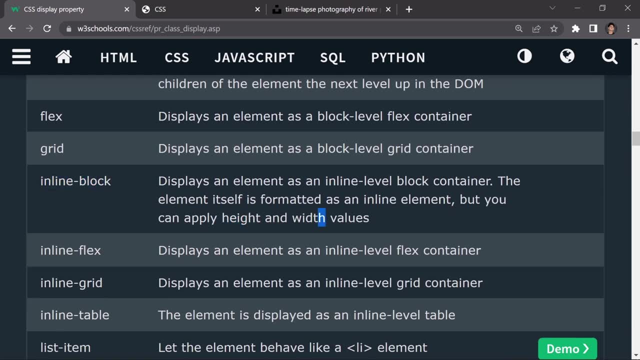 hide and with to it, in just an inline to it. so uh, just if you just write like inline, so height and width will have no effect on that. but on the other hand, if you use like inline blocks, so we can use height and width on it. so uh, instead of writing like lorem 10 and stuff. so i'm going to just try. 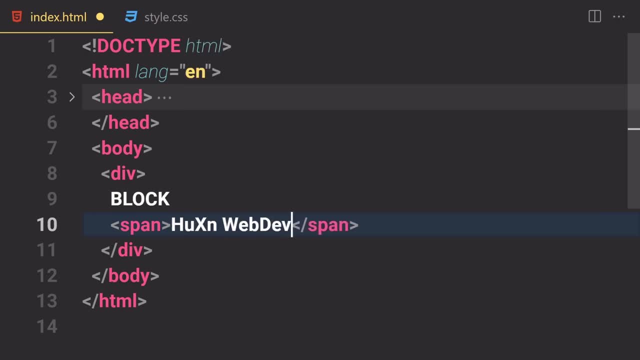 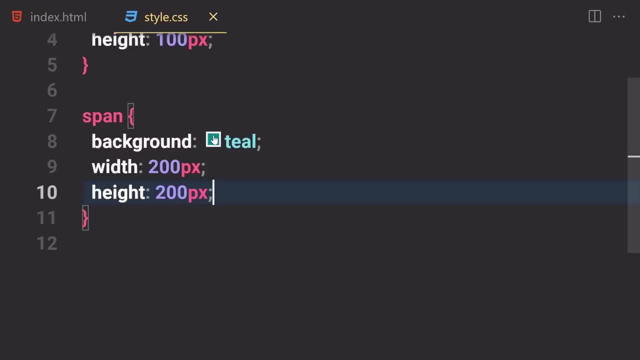 like uh, i don't know my name- like who's in web dev right here and now, if you save that and if you check it out. so here you can see, we have like this inline tag right here and, as we learned, that we cannot provide a width and height to it, but we can change. 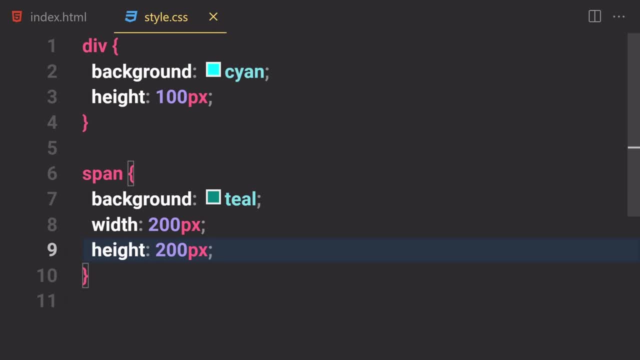 the display property of it. so how can we go about doing that? so i'm going to just provide, like, a display of inline. if we save that, here you can see it's by default inline. so if i just write instead of inline, i'm going to provide an inline block and if you save that and boom, here you can. 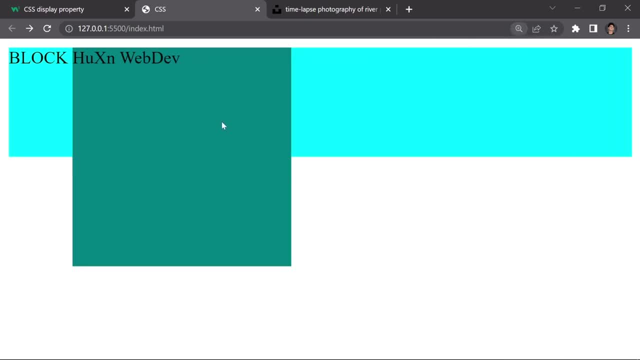 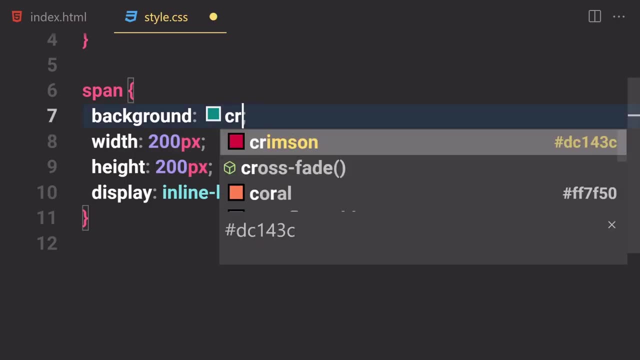 see it did took like a hundred percent of width and hundred percent of- not hundred percent to be precise, but 200 pixel of width and 200 pixel of height. here you can see that we can change the color to be like crimson and cell file, and this is how it looks like right here. okay, so these are. 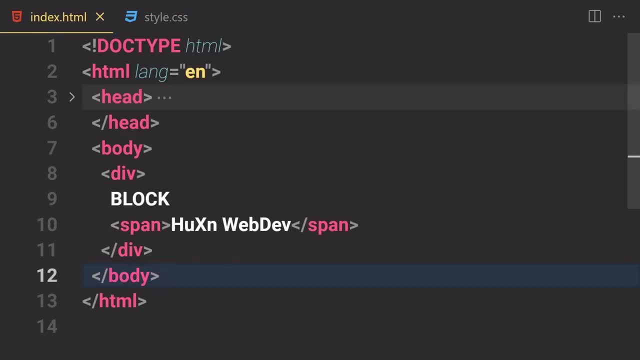 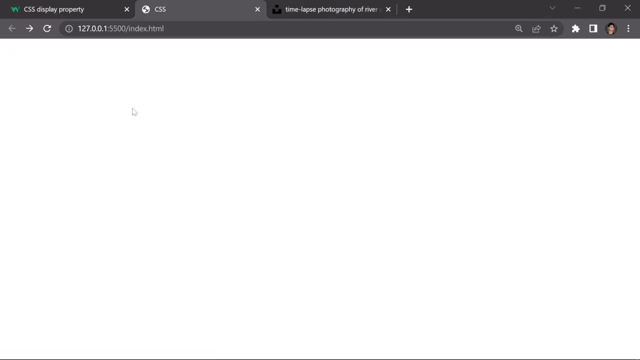 just a man and a subtle difference between all of them. so now let me just show you a few more things about inline and block one. so i'm going to remove all of this code. so now that you know the differences between inline, inline block and block level element, so here we have like a div and this: 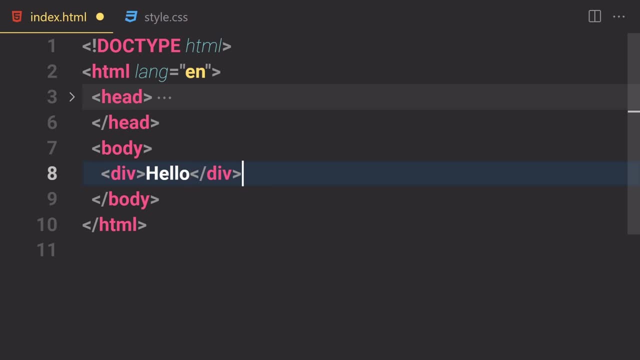 div is like: uh, if you just write hello and this div is now by default a block level element, if you just write it like block, and now if you save that, and here you can see, we get a block right here if you select that div. and now let me just write a. 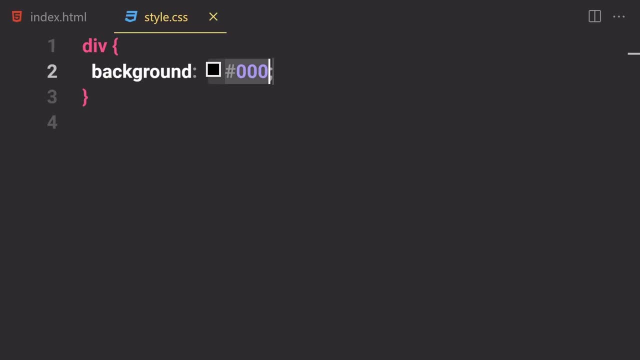 background color to be like, uh, i guess black would be fine. you know, not black, but just a teal would be fine. so now we have this block level element, but we can also make that as an inline level display. so how can we do that? we are going to be just writing a display of inline, okay. and now if 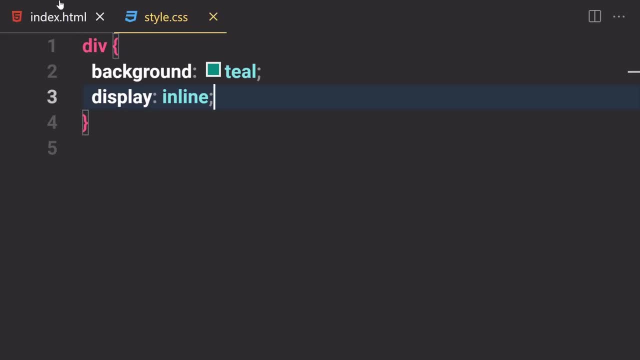 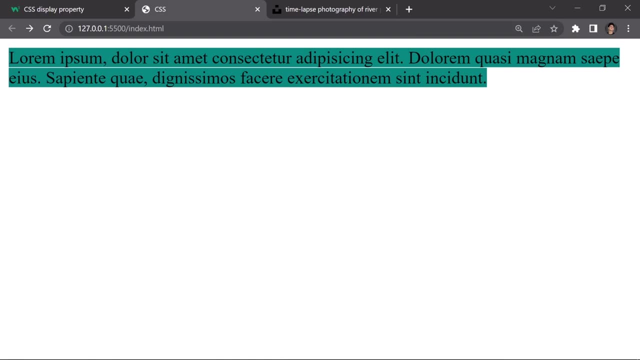 you save that and here you can see, it's not taking its entire space, but instead, if you just write something like a lorem of 20 and if you save that and here you can see, it will now take just the content space right here. okay, it will not take the entire space, but just a content space. why is 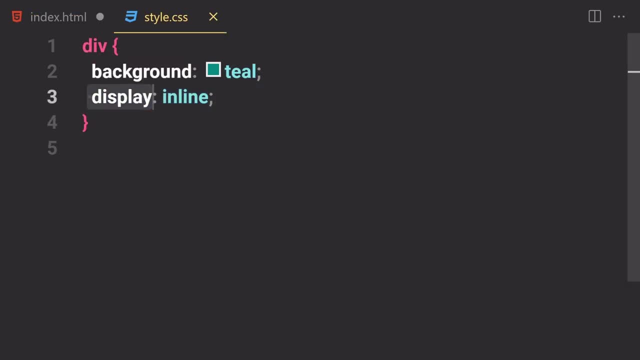 there. that's because we just set the display property to inline right here. okay, so we now converted our block level property to be display inline. okay, so now, if you save that, and now let me just write a block in here, so now we converted that to, uh, inline one. but instead, if you just write, 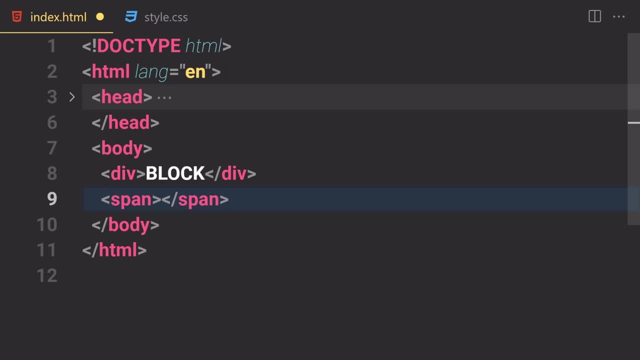 like span in here. so we already know that span is an inline tag and also image is an inline tag. the anchor tag is an inline uh display by default. so these three are by default display of inline. okay, so if you want to change like, let's suppose you want to just write like uh inline in here and 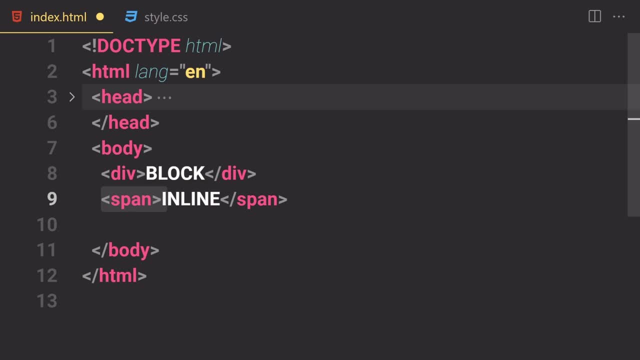 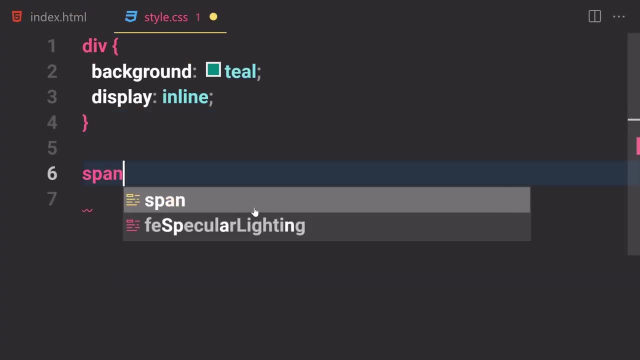 now if you want to change this inline property to block, so how can you do that? if you save our file and here you can see, it will be inline by default. let's just style that a bit. i'm going to select my span in here. i'm going to provide a background of crimson. 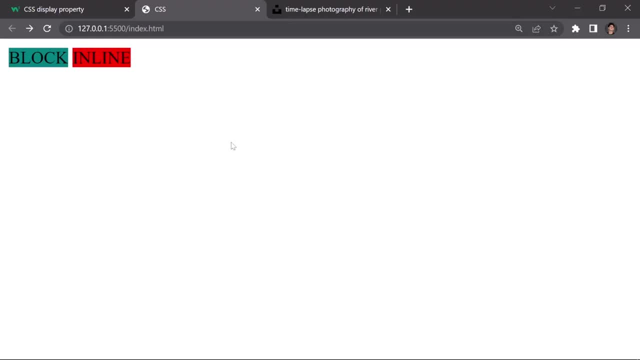 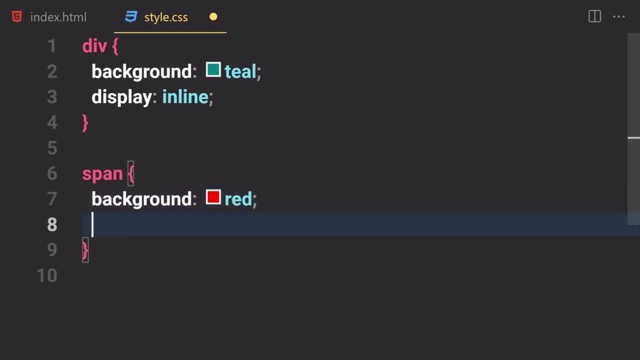 uh, crim or you know what, red would be fine, not a crimson. so save it and here you can see it will be. it will also take, uh, just a content space, but it will not take the entire space. but if we just write the display to be block and if we save that and boom, it will now take its entire space and it. 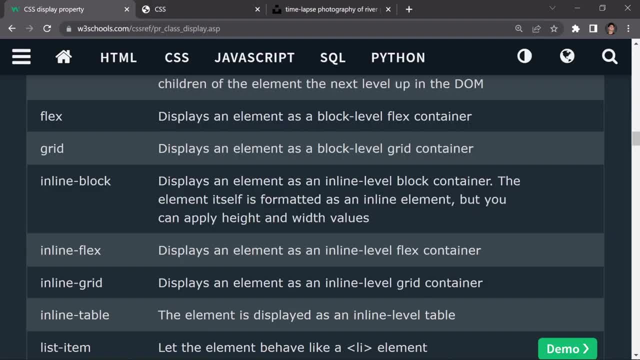 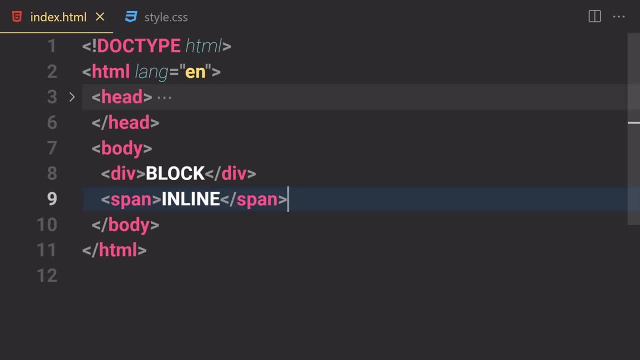 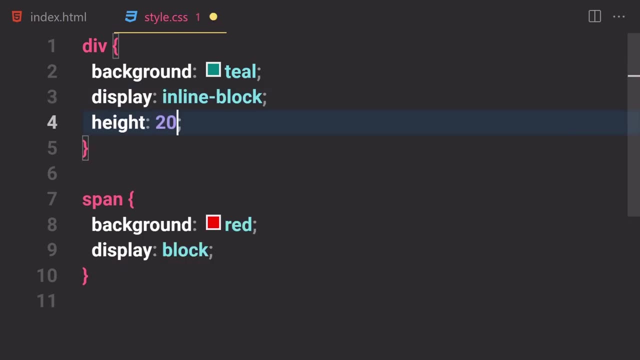 will be in now in new line right here. okay, as we learned that inside these instructions and this is what's happening right now, and so these are that too, and we can also just write an inline block if you want to, so we can also set that to like inline and then dash block. we can also provide a height of. 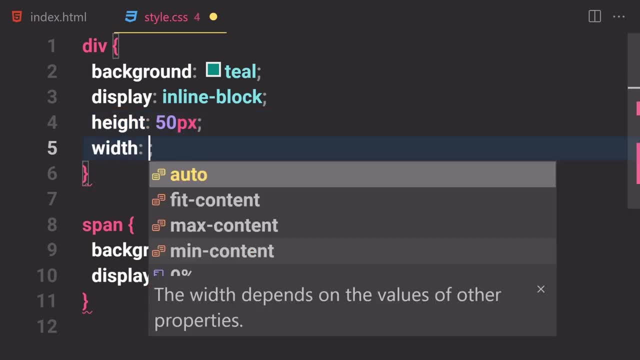 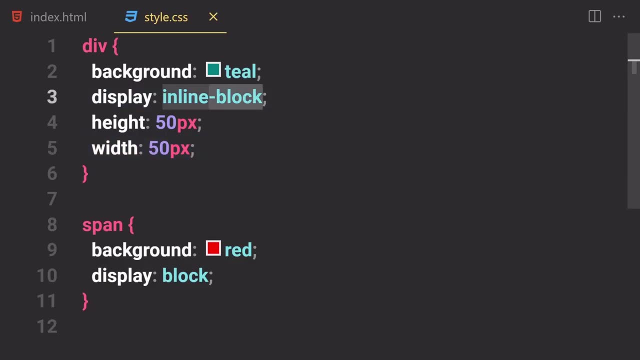 like not 100 but 50 pixel, and also the width of like 50 pixels. so now, if you save there and now it will take this width and height. on the other hand, if you just change that to just an inline one, not inline block, and if you save there, it will not work like this height and width will. 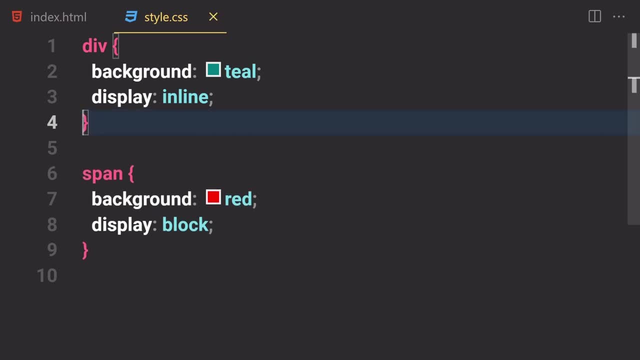 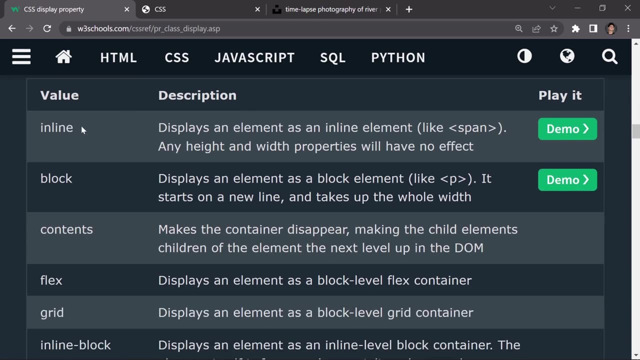 not affect it okay, so i'm going to just remove that anyways. so that was it about a display property. we have three kind of displays, not just three kinds of displays, but in this section we just learned about three kinds of value of display, like inline block and inline 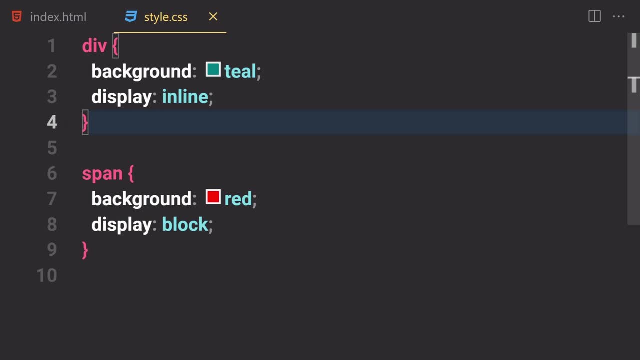 line block and we also have another one which is known as a display of none. so now let me just show you that real quick. so if you just write a display of none, it will just entirely remove that element from our dom. if you just write display of none, save it and boom, that's gone. we just kind of 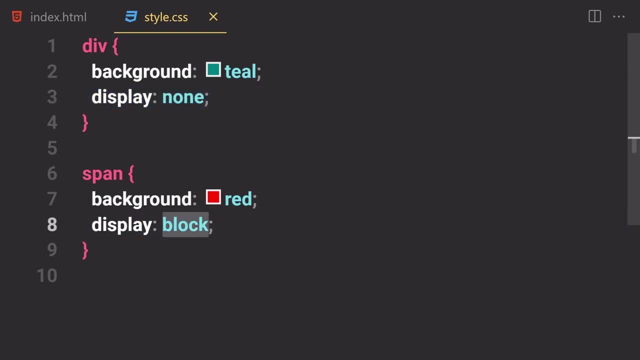 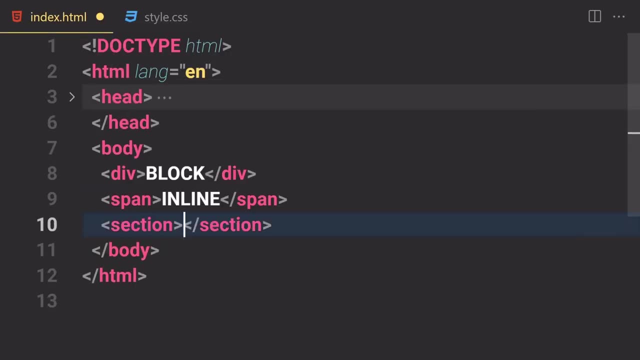 deleted that element from our dom. and now if you just write display of none in here and if you save that, boom, this one is also gone. if you just write something else, like maybe section we have a ul, then we have a ally, then we have an anchor tag and we have all of these stuff right here. and if we save, 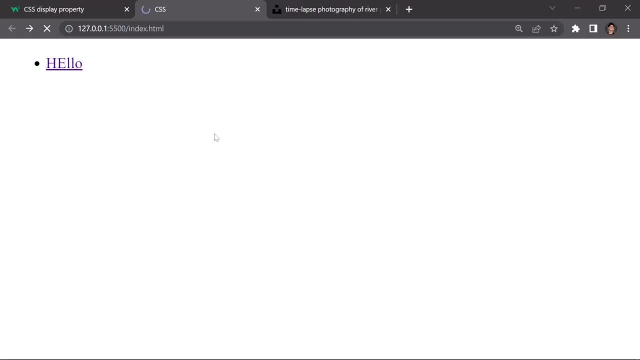 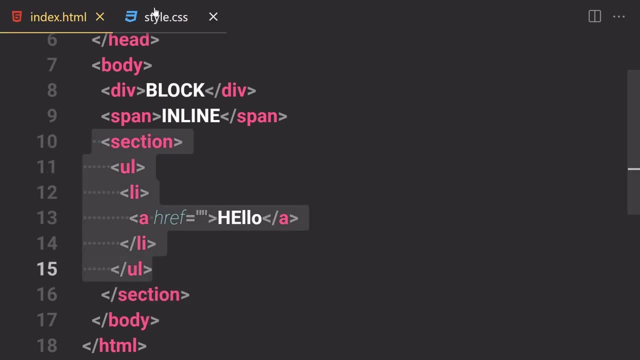 and we get. just come on, let me just write a hello and we have this hello and now if you want to provide display of none on this section, so it will now just remove all of this content, okay. so if you want to just select this section and we want to pour a display of none on it, and if you save that, 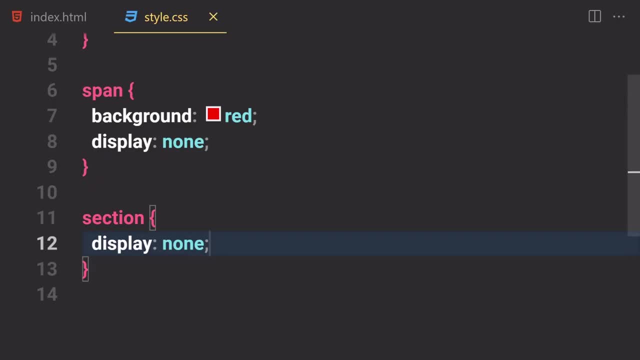 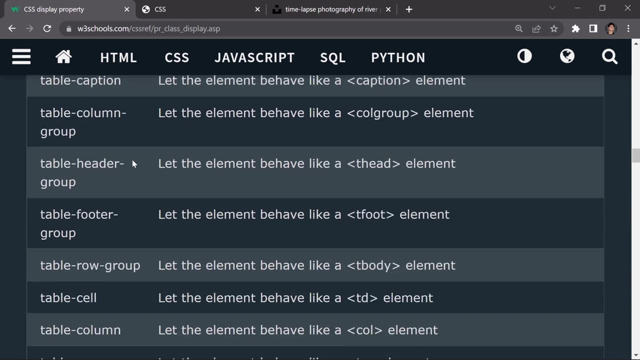 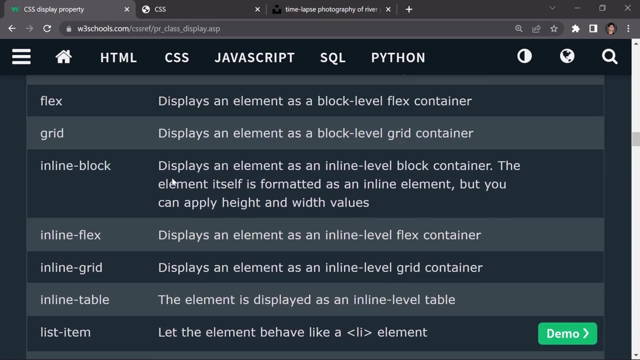 and boom, everything is gone from our dom. so this is how we can work with that. so we just learned about display of inline block, inline block, and we also learned about a none, uh, okay. so here's another thing that we learned about in the upcoming sections: uh, flex, which is my favorite. i really 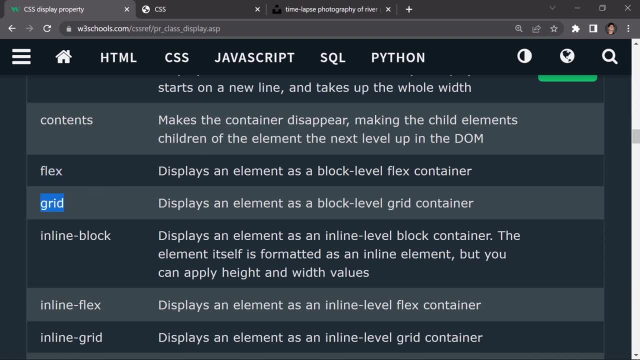 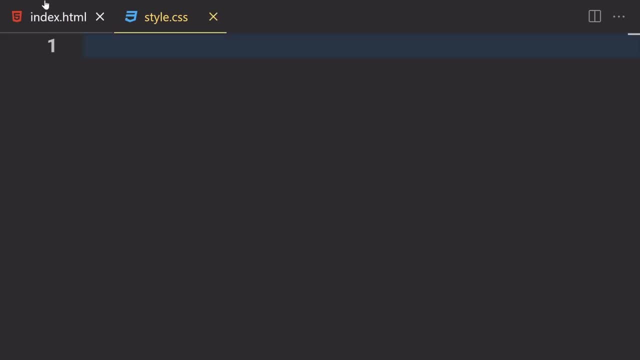 love flex, display of flex, and then we are going to be also learning about a great one as well. so congratulations, for now you have tackle, like maybe 50 of css, so we have a long road to go still, so i'm going to remove all of this coding from here and now. we have totally a blank screen, right? 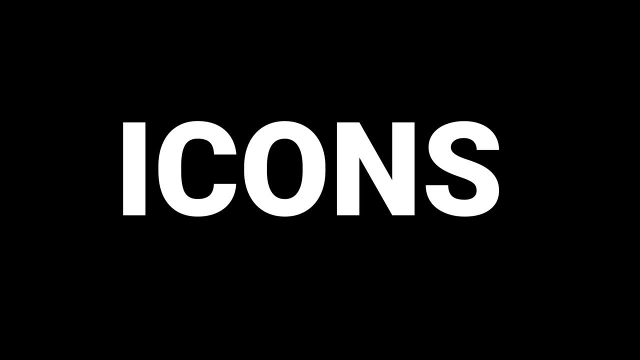 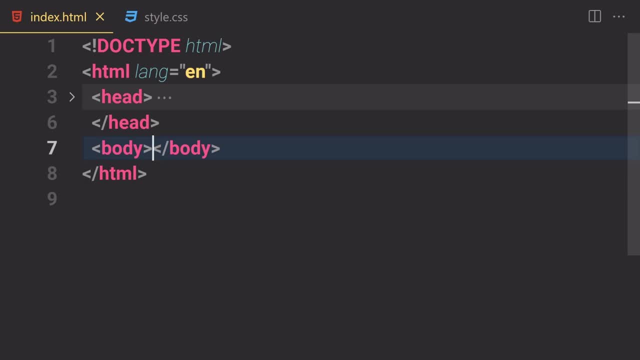 now all right. so now let me just talk to you about how to use flex display of inline block. inline block and we are going to talk about a font. awesome in some cases, in your website, you want to use some sort of a font, like some sort of emoji, not a font. 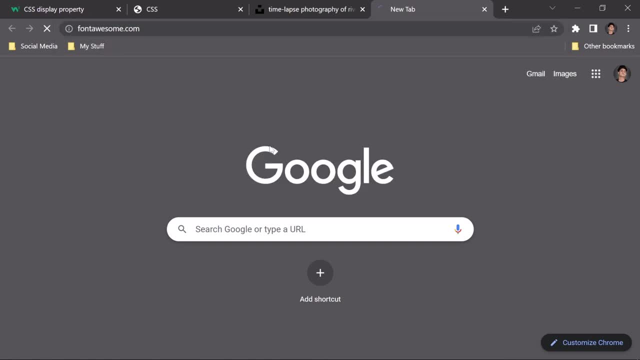 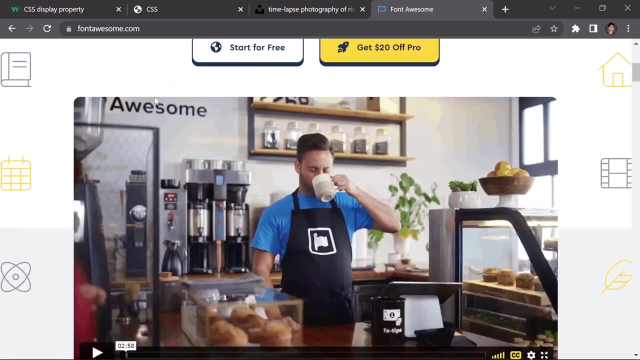 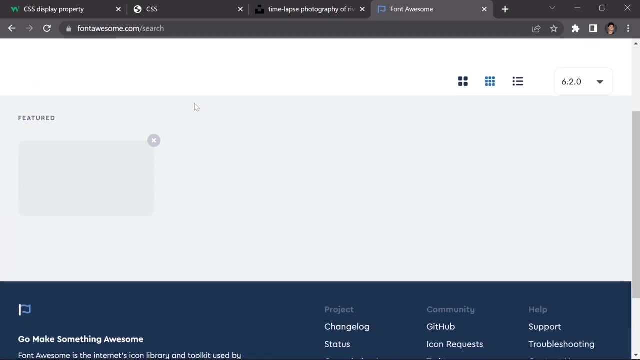 but emoji to be precise. so if you want to get there for that we have to just go to the font awesomecom website. so if you go there, so in this website we can find lots of cool svg icons and stuff. some of them are free and some of them are paid. so if i just click on the search gear icon. 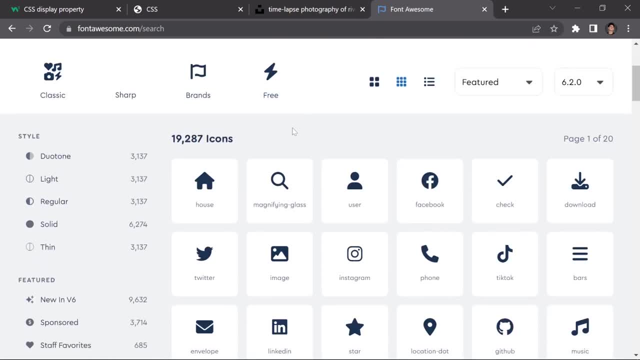 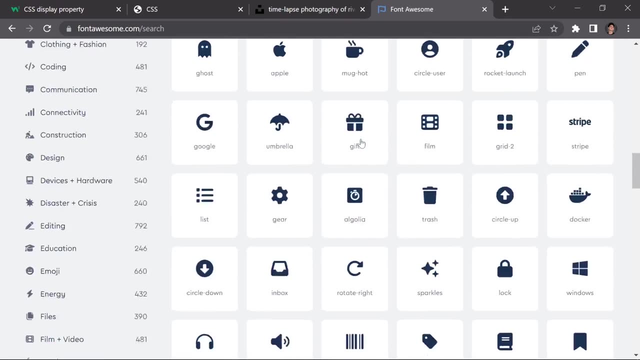 so it will now give us all of this library, okay, so which we can choose a lot of font from, like we can choose home, we can choose magnified glass, user facebook check, download, and there are like countless of fonts right here and you can also check the categories if you want to. you can also. 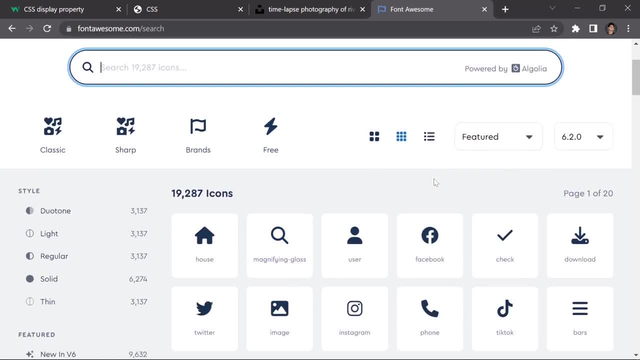 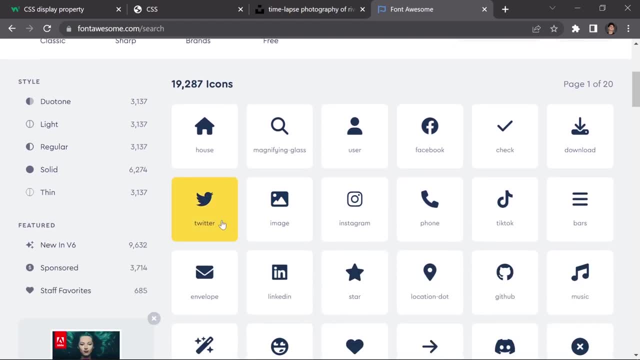 download these font into your machine, but we're not going to be doing that. so suppose, if you want to use, maybe like uh, this twitter font in your um social media icons or whatever. so if you not, a why am i saying font all the time? but social media icons, to be precise, not font, if you want. 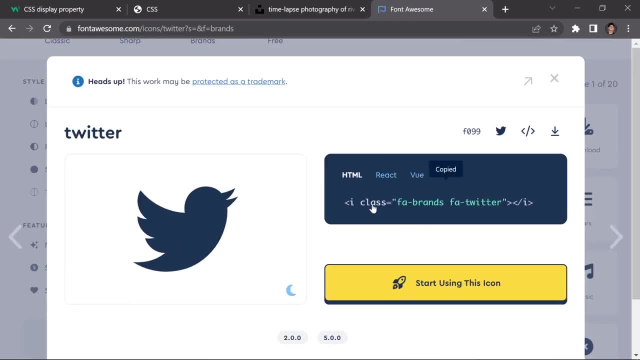 to just select this trailer. so i'm going to click on there and now we can just copy there and we can paste it inside our body tag. but it will not work. why? because we have to get a cdn of this font awesome library. so to get there. so first of all you just go to the cdnjscom, and now i'm going to. 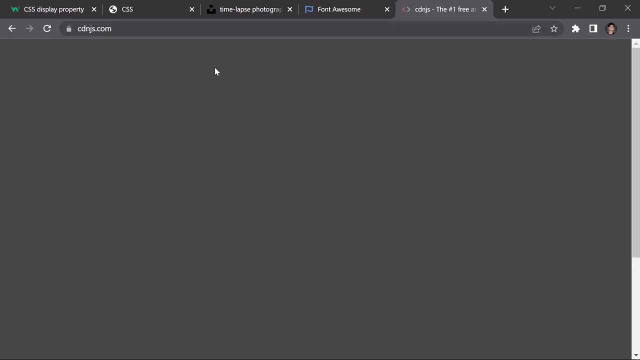 hit enter right now, so it will brings us to the cdn uh js page, which you will see just in a second. so it takes a little bit of time and it's a little bit weird website. you will see that just in a second anyways. so here you can learn more about this. 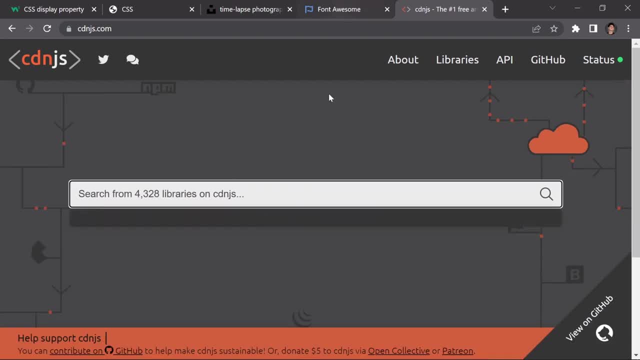 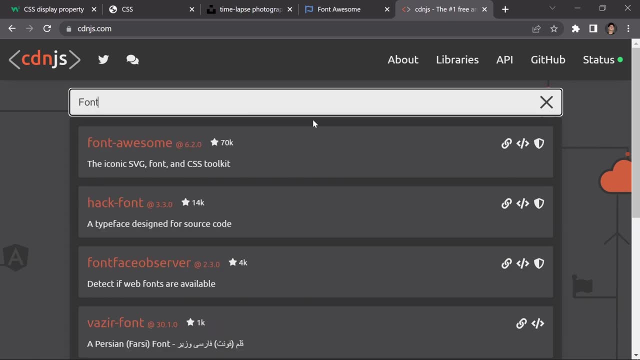 website if you want to. but in my case i'm just interested in font awesome. so what do i have to do? i'm going to just search for font. oh my goodness, here you can see the weirdness. so if i just write font, then i'm going to click on: okay, so we got a font awesome cdn right here. then i'm going to just 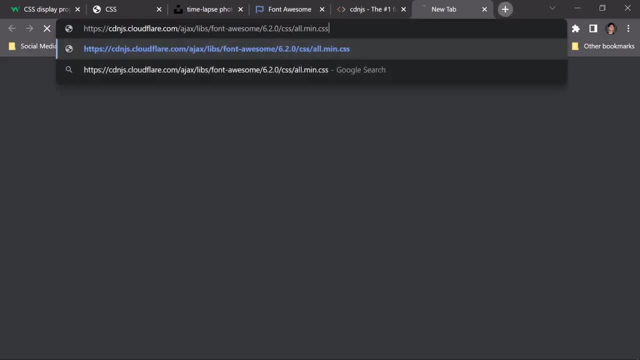 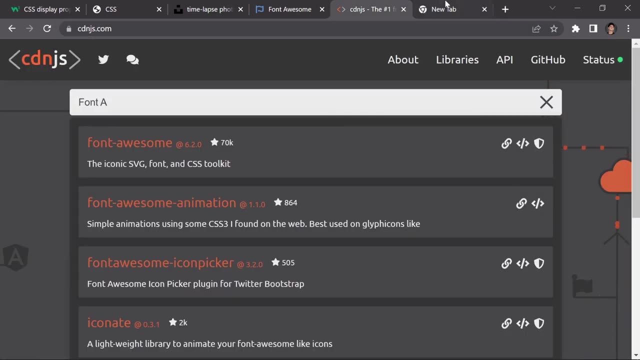 click on this copy url. if i click on this copy url and here i paste it, so here you can see, it will not use the url, we are not interested in it. so i'm going to just click on this copy url and that one we are interested in copy the link tag. so if you just copy that and if you paste it right, 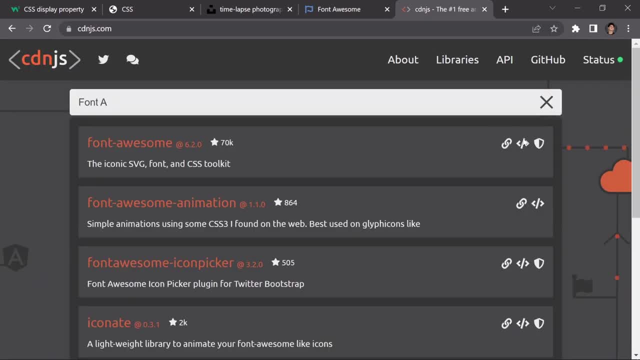 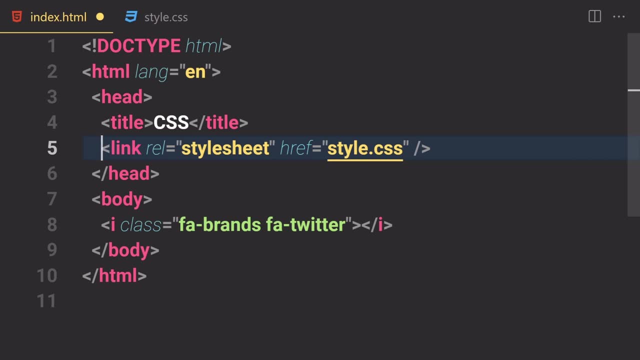 here and here you can see. this is how it will look like anyway. so now i want you to just click on this copy link tag and then open your head area and underneath your uh link, right there or not underneath, above your link, because we want to render, or not uh above. let me just put that. 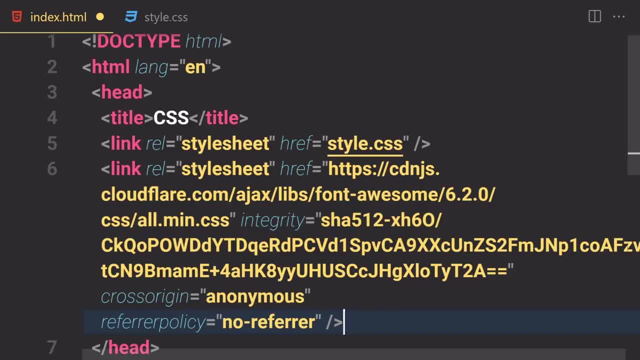 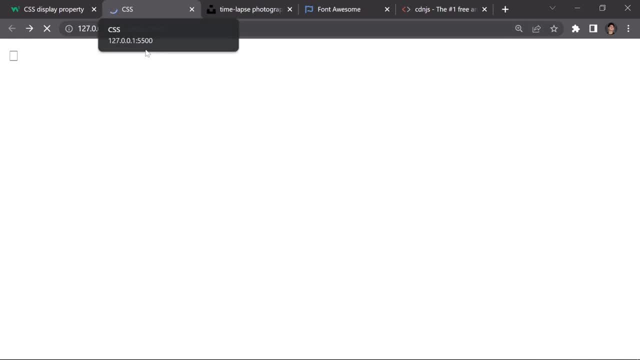 underneath. so let me just remove that and put it underneath this link. and now if you save that, and now if you go to your css file and here just wait for a second, my internet speed is just a little bit clunky. okay, it's not game. come on, give me that awesome font icon. so 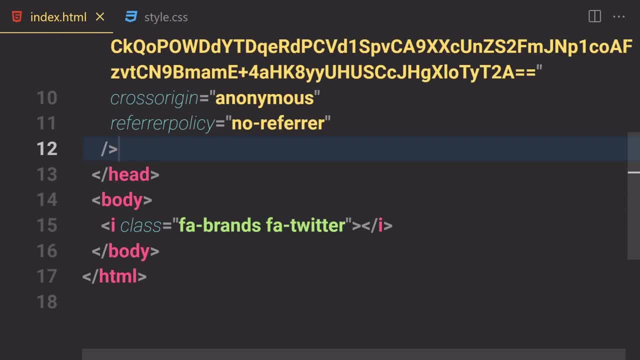 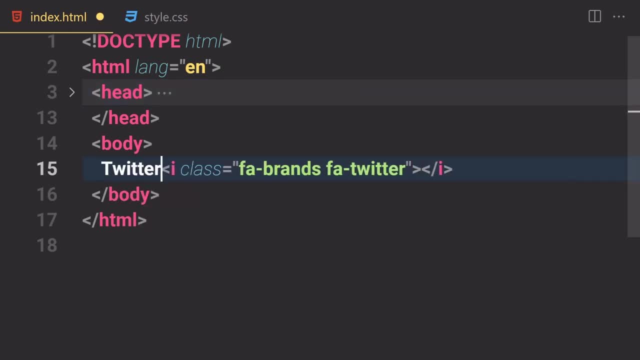 all right. so here you can see: unlock uses this twitter icon. you can write your text inside there. but before we do, i'm gonna hide this head area and we can just write like twitter and save it. and this is how it will look like: we can get a car, we can get like instagram heart. 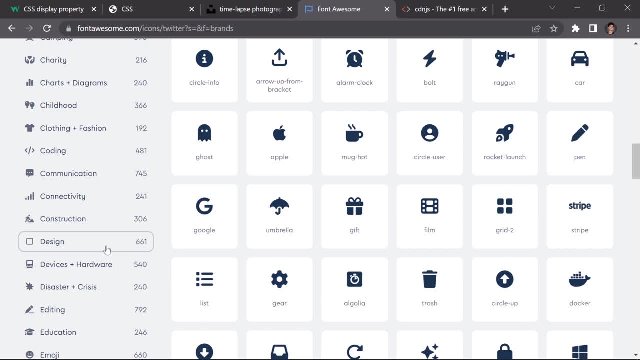 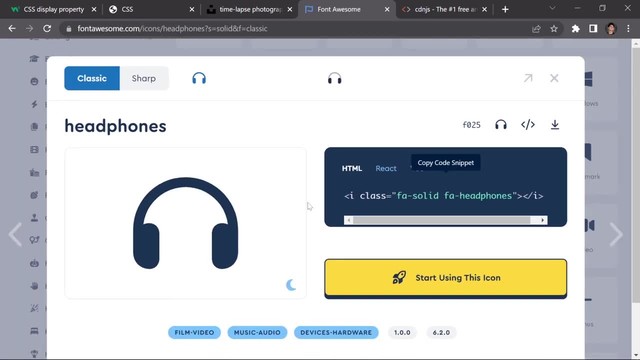 we can just play around with that and there like countless font construction, design, device and hard drive and stuff like that. in my case, i'm really a big fan of a headphone, so i'm gonna just click on this um link. so if i click on it so it will just copy it to my clipboard if i want to. 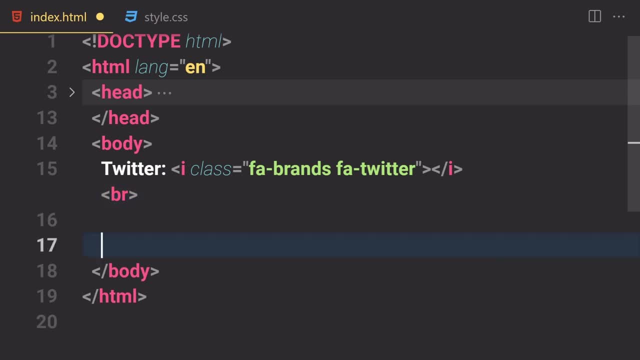 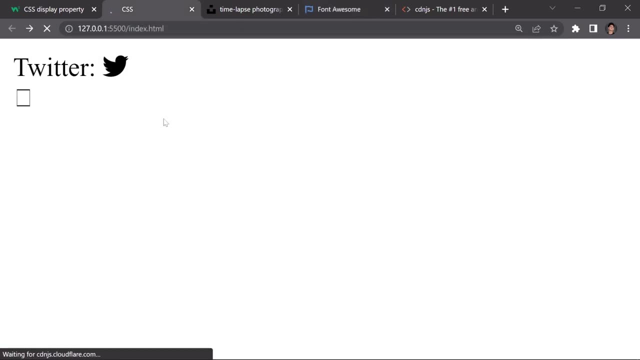 put it right here. so what do i have to do? first of all, let me just write a br for myself, and i'm going to just write. like you know, i'm going to paste it right here. so if you save that and now here, you will just see in a second that we will get our phone and my internet speed will go down. 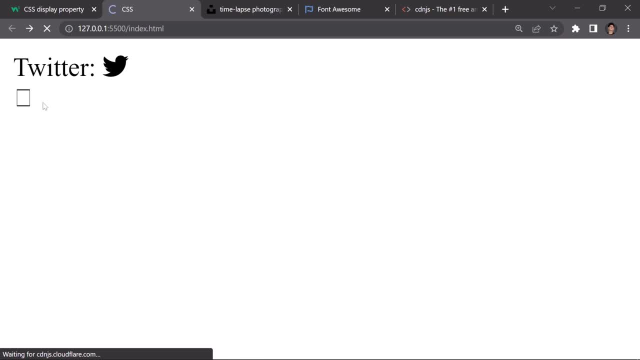 my internet speed is so slow, so that's why we have to wait for it. and now, here you can see. finally, 24 hours later, we get our headphones right here. so this is how you can work with that. and now let's suppose, if you want to like, change the color of them to like something else, like in. 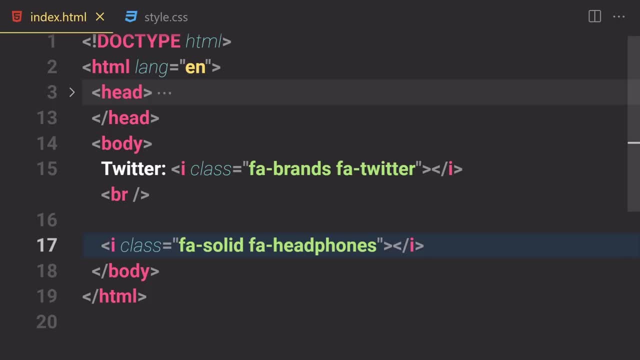 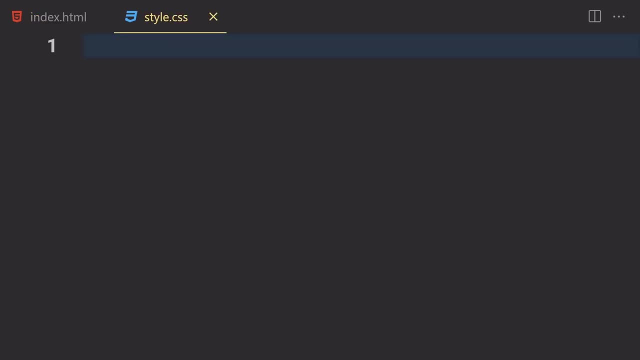 my case, i want to change this color to be like blue. so what do i have to do? i can either select this class or this class. so let me just select this fa brains and i'm gonna first of all write a period and then i'm gonna provide this fa brains in there and i'm gonna provide like color of maybe. 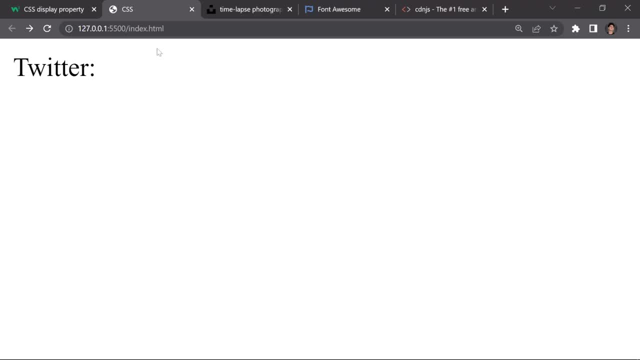 blue. and now, if you save that and we have to wait for it one more time, come on. and now, here you can see, the color is changed to blue. i know it's not a twitter blue, but it's pure blue. we can also change these headphones to something else, so, uh, i'm gonna just copy this link in: uh, or this class: 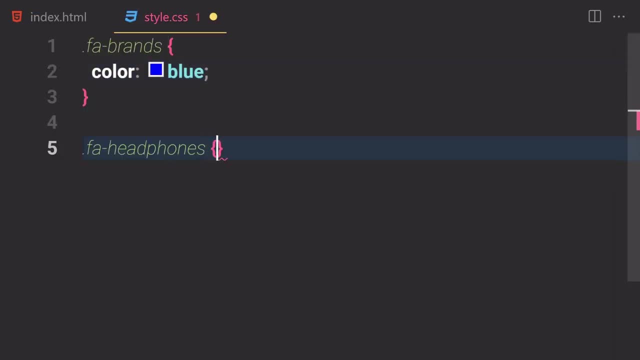 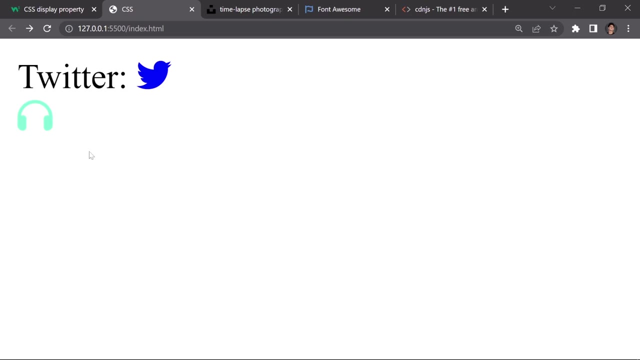 to be precise, and now let me just write a dot and then let me just paste in here and color would be maybe this kind of a green ish color, and if you save that and here you can see, the color is changed to this kind of a greenish. 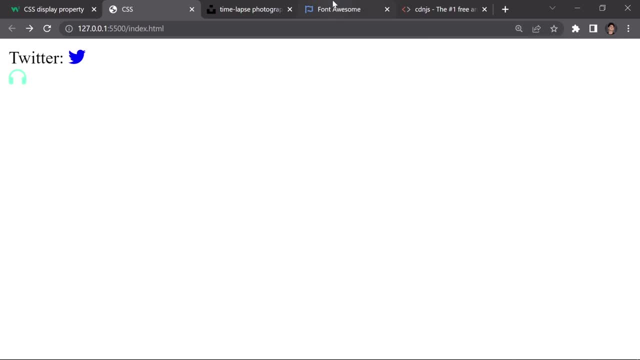 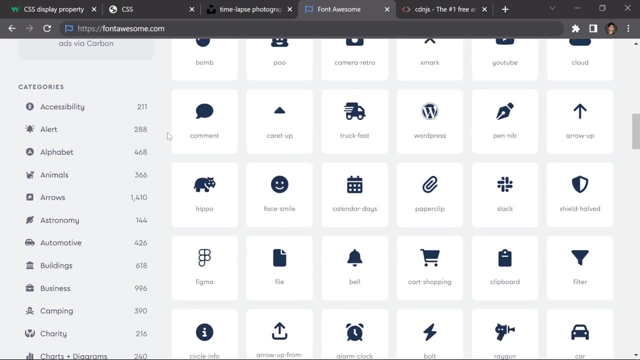 color. so this is how you can work with a phone. awesome. first of all, if you want to get a phone, you just have to come to this website, which is just a phone- awesomecom, and then click on the search gear or you can learn more about their phone. awesome. if you want to, you can go as a 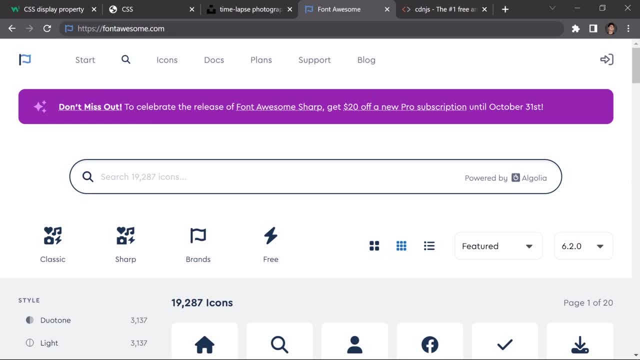 pro version if you want to, but i'll not recommend you to do that. and now, if you want to get a excedian, there would be some place to get excedian, but i'm not sure where is that located. so i just click google search and we get like cd and js and i just search. 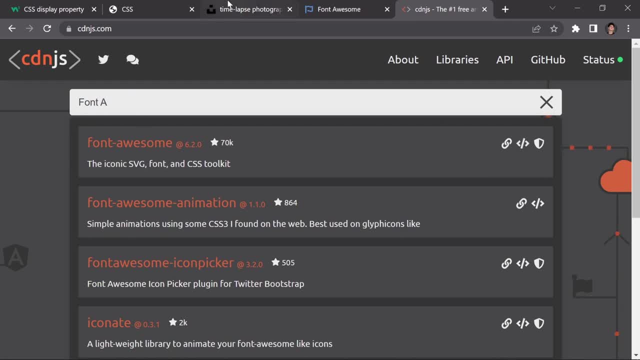 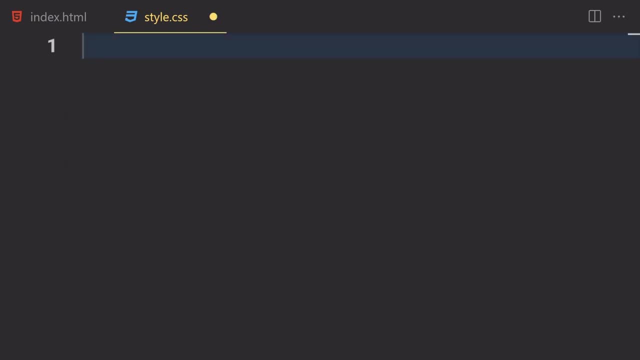 for a phone- awesome. and then click on this copy link tag and we just put the inside word head area and boom, everything is working the way we expect to work. so that was it about uh font, awesome library. i just kind of want to show you that i'm going to remove this one and i'm going to also. 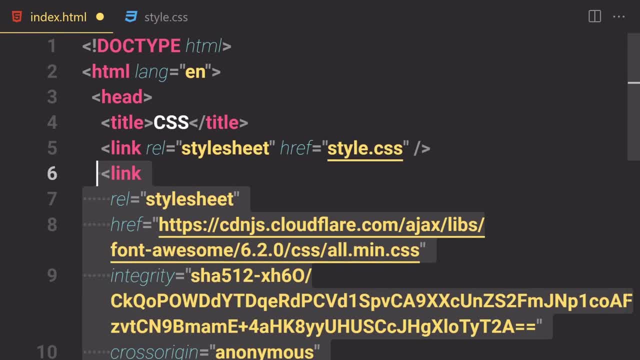 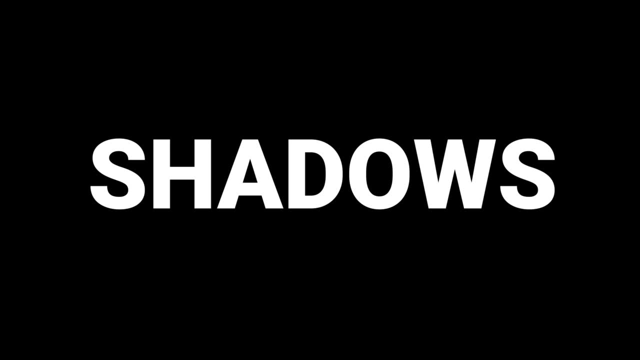 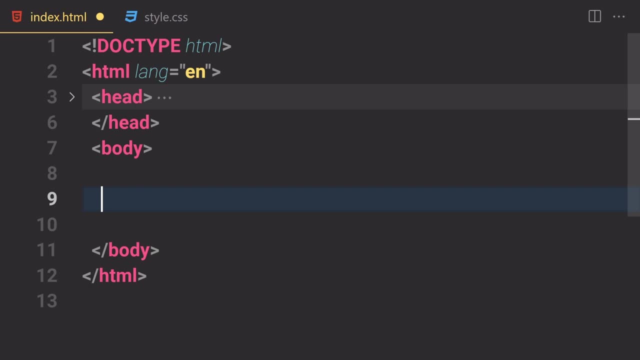 remove this link from here. okay, say bye, bye to them and let's just hide this head area. and now we are totally good to go. so the next topic i want to talk to you about is something called box shadow and a text shadow. so how would we work with the shadows in css? so first of all, let me just write a div, and we are not going. 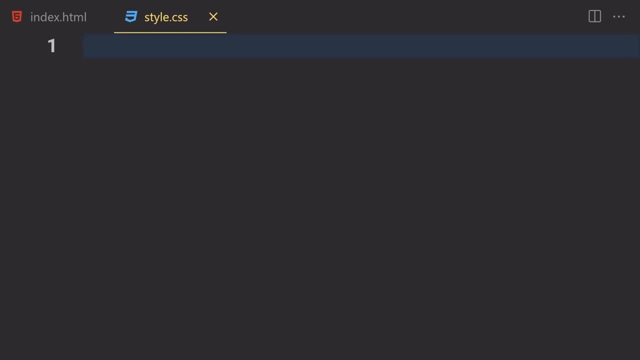 to be writing any content or whatnot. so if i just save that, now i'm going to have to go to my css and let me just select my div, and inside this div, i'm going to first of all give him a width of like 200 pixel, and i'm going to also provide a height of 200 pixel, and background color will be like: 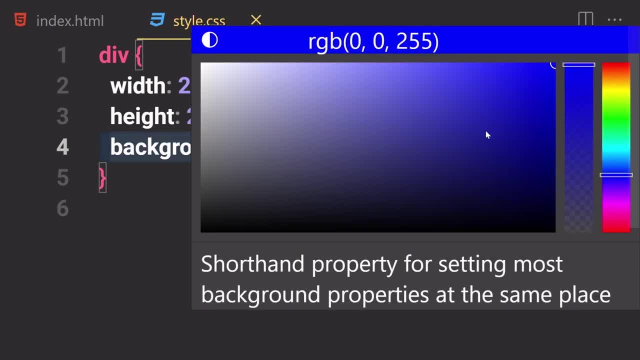 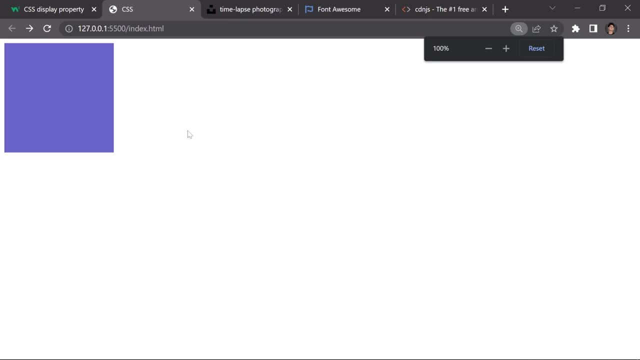 kind of a blue color or you know what. let me just change the opacity of the. i'm not a fan of pure blue. so if you save that and you already know what we will get inside our browser. so this is what we get. so now, if you, 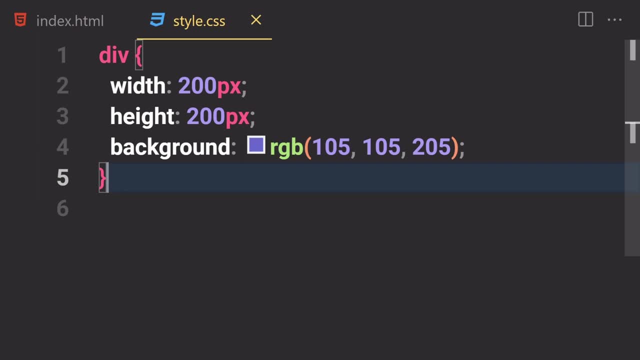 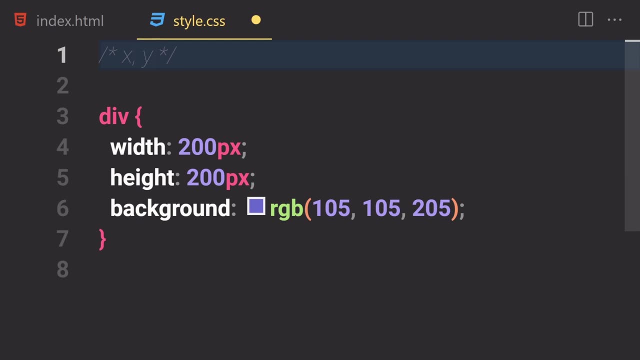 want to provide a shadow to this box. so what do we have to do? well, there is just a syntax of a shadow. first of all, we have to write a value for the x-axis, then we have to write it for y-axis, then we have to write it for a blurness and also for the color. okay, so this is just a syntax of: uh, if 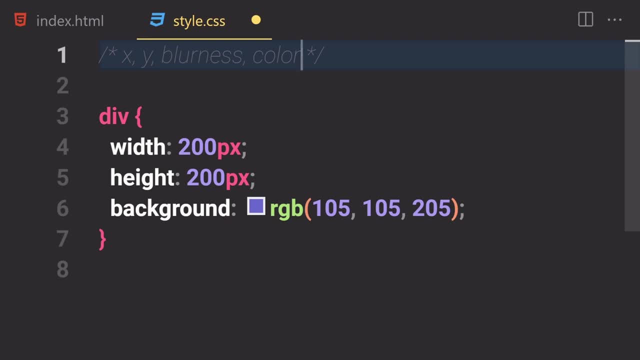 you want to work with either a box shadow or a text shadow, and then you can also create a text shadow or a text shadow. so you just use this syntax. so first of all, if you want to work with the box shadow, so we just have to write a box shadow property in here and now. here we have to first 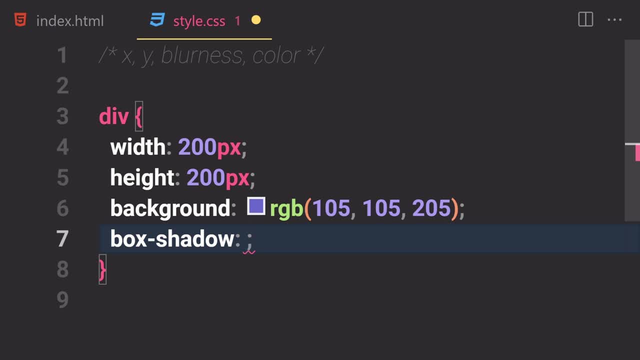 of all, write a value for the x-axis. so how many x-axis we want? we want them to be like 10 pixel- a lot. and then we want them for a y-axis- 10 pixel one more time and blurness will be like 20 pixel. 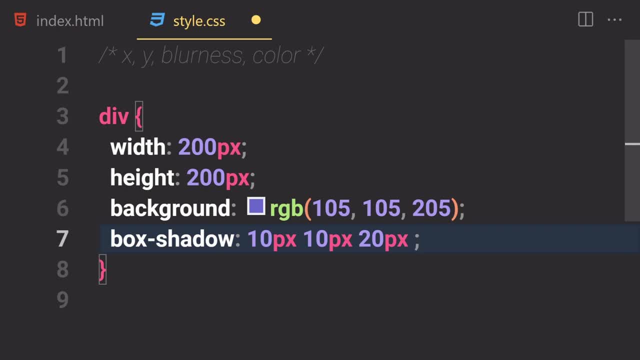 and the color will be by default. the color will be black, but we want them to be like orange maybe. and now, if you save that and here you can see, it will now put out this orange kind of shadow. right here you can increase or decrease the size of air, so i'm 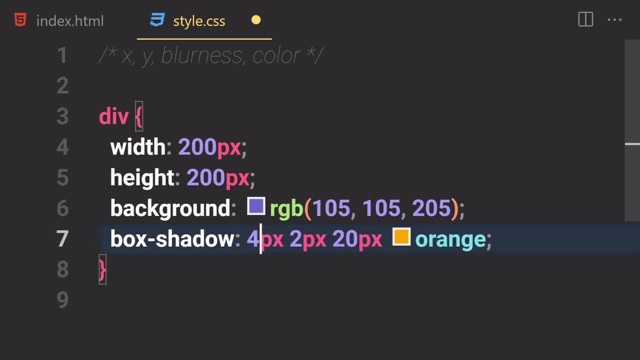 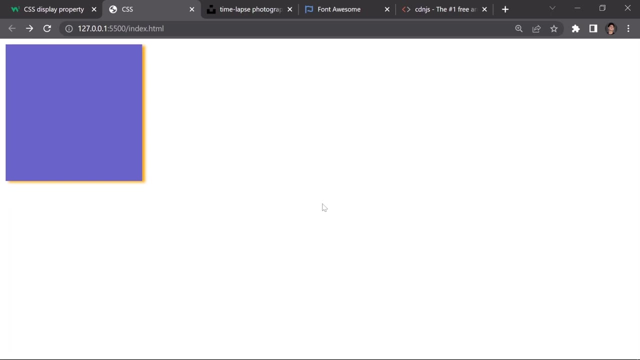 going to just stick to like two and four. so if you save that, and here you can see, this is how it looks like and we can also change the- what do we call it blurness. so if you save that, and this is how the blurness will look like and you know what, i'm going to just write it four like, so uh-huh. 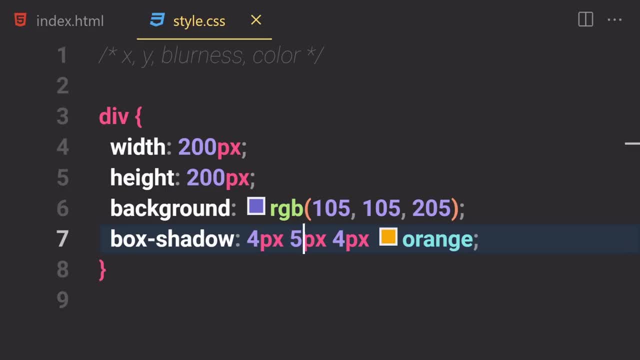 let me just change that to five. yeah, this is looking cool so you can just play around with it if you want to. but i just kind of want to show you is that how you write a shadow for your box or for your text? so if you want to write it for text, you know what i'm going to remove this. i'm. 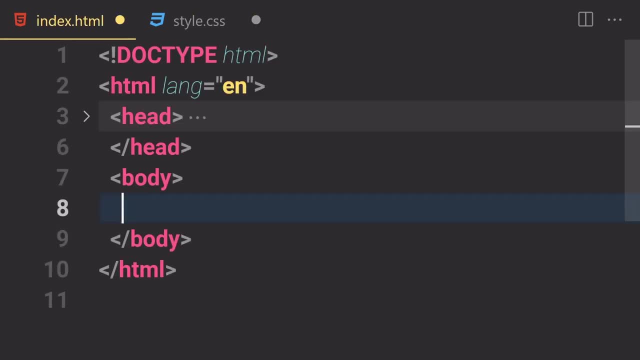 going to remove this div. i want to show you something cool and i'm going to also remove this div. i'm going to write h1 of my name, like huzen web dev. so now, if you save that, now i want to go to my css, i'm going to select my body and i'm going to provide a background color of totally. 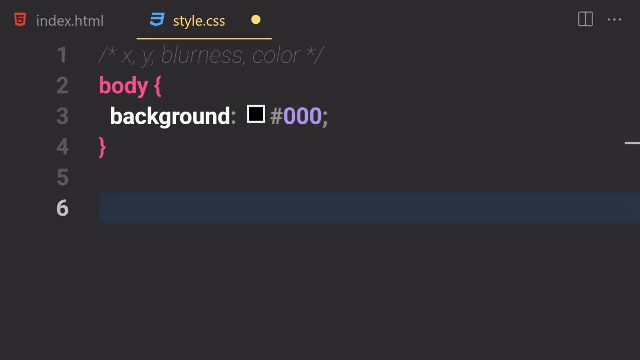 black, so save it. nothing will show up right here, okay. so now let me just select my h1, which is this div, right here, okay. so what do i have to do? i'm going to just provide, like a box shadow of i don't know, two pixel, two pixel, two pixel for the blurness, two pixel for the x-axis, for the y-axis, then for 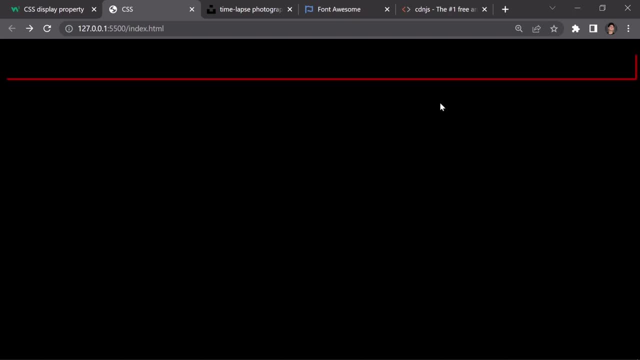 a blurness and i want them to be like red. so if you save that and we cannot see, okay, so i'm just using it for box shadow- it should have to be a text shadow. and now if you save our file and this is how it looks like right here, okay, so i'm going to just bump up the size, so i'm going to use font. 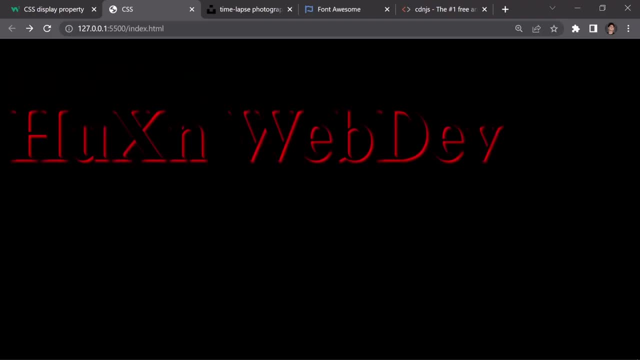 is to be like four or you know five, from what we find, and if we save that and this is how it looks like, and what else do you have to do? i'm gonna write a text line of center and, boom, look at this name. i mean like we can also provide a margin to the top and we can make it clear as we like. 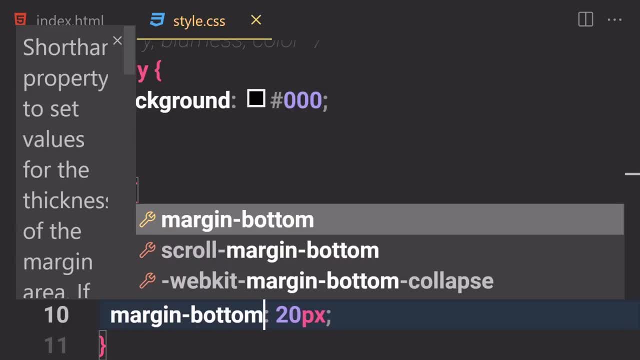 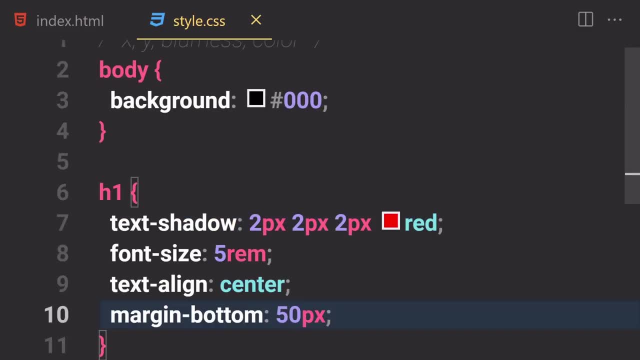 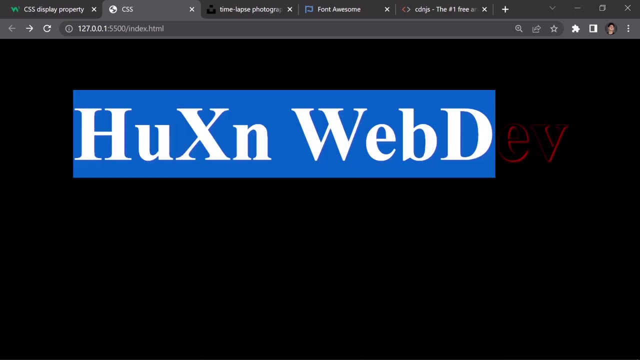 okay, so not for the top. uh, i'm gonna provide for the bottom, save it, and instead of 20 i'm gonna put like 50, and this is how it looks like we can play around with the margin. uh, not a margin, but x-axis values like one, one and two. blurness would be fine and you can play around with that and you. 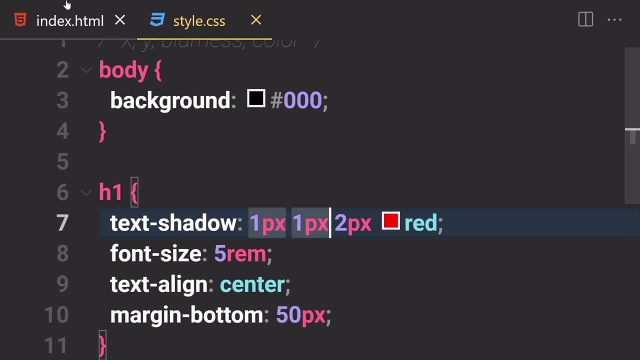 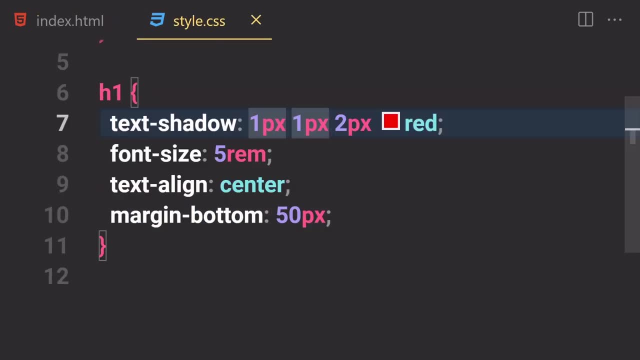 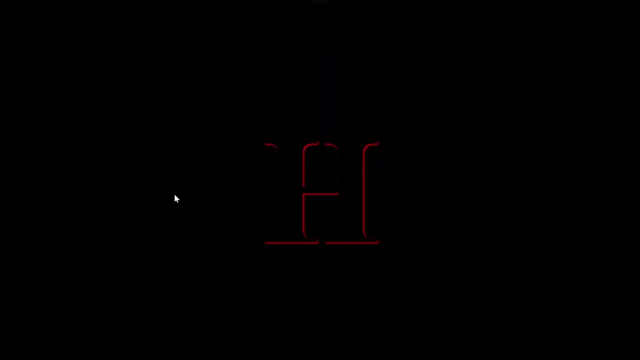 can get these kind of effects if you wanted to. okay, we can just go with h. i'm gonna remove all of them and put it inside there and this is how it will look like. but i'm gonna have to increase the font size to be like 10 ram severed and boom. this is how it would look like kind of old school horror. 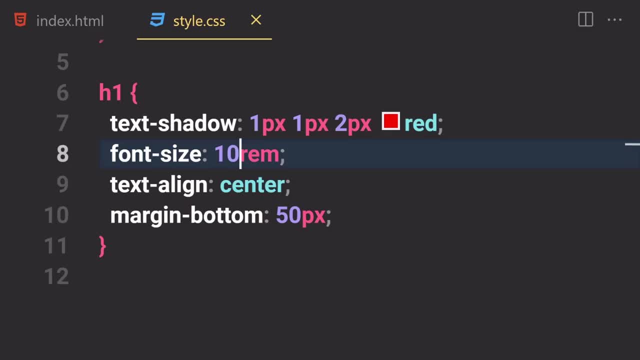 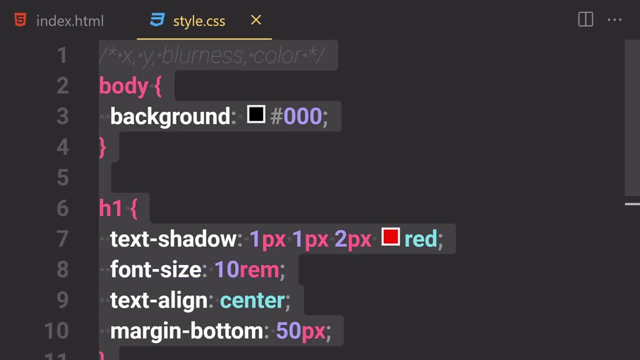 movie, uh, headings anyways. so you can play around with that if you want to, but i just kind of want to show you how you would work with that text shadow and a box shadow. so now, what do we have to do? i'm going to select everything and remove it, okay, and i'm going to also select this h1 and 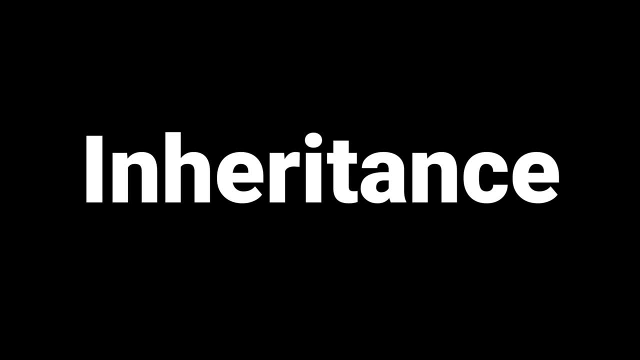 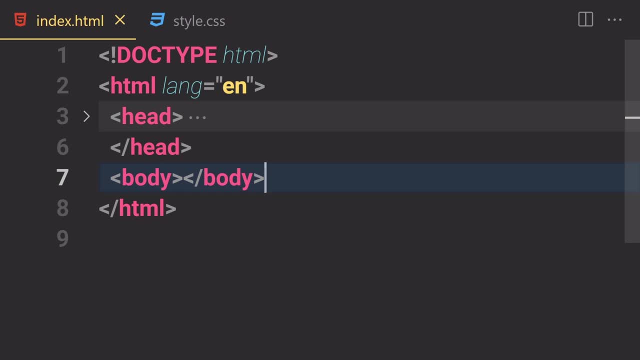 remove it so that we can get a clear screen. all right, so now we will learn about box shadow and text shadow in css. now the next topic which i want to show you is something called inheritance in css. so inheritance is like not a hard topic to learn, but it's kind of like a theoretical topic. so you 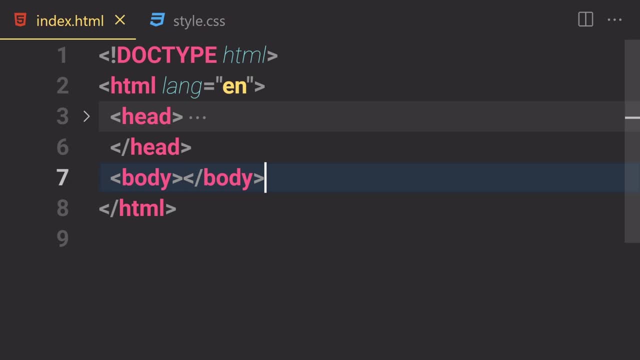 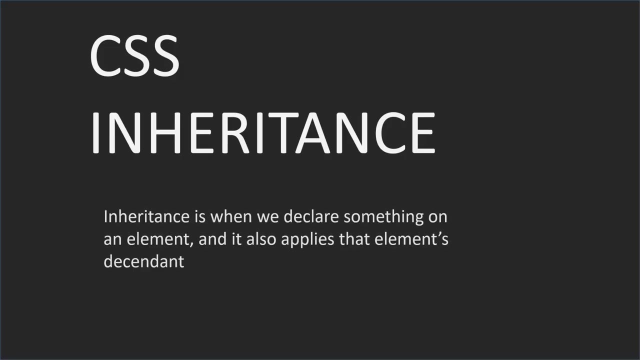 watch some slides and i can totally promise like my slides are not that much uh boring, and i'll see on the slides, all right. so what is the css inheritance? a css inheritance is when we declare something on an element- and by something i mean, like styling on the element- and it is also applied. 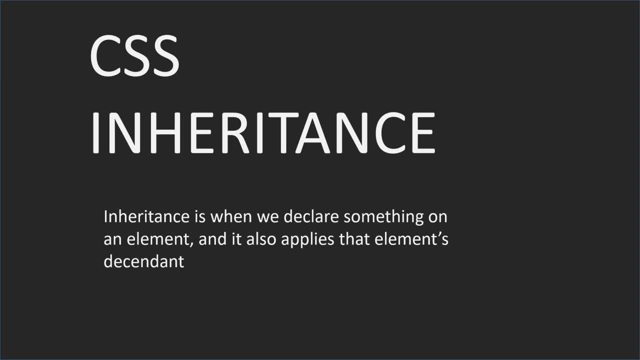 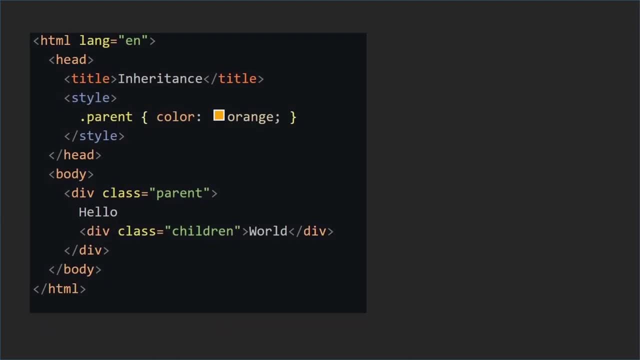 to the element descendant. so what do i mean by all of that? so now let me give you a quick example, and then you will get to know what i'm talking about. so here i want you to just notice this code. so we have a structure and inside a body we have two divs. so the first div have a class of parent and 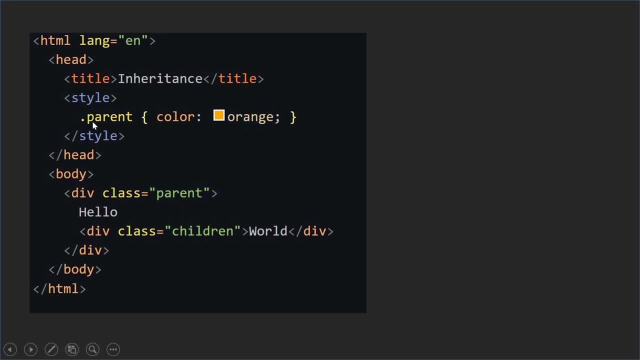 the second one is a children, okay, and inside a parent. we are now selecting first of all the parent, and we are just changing the color to be orange. so what do you think is going to happen? does this children will also be inherited, or not? well, obviously it will be inherited. so what do i? 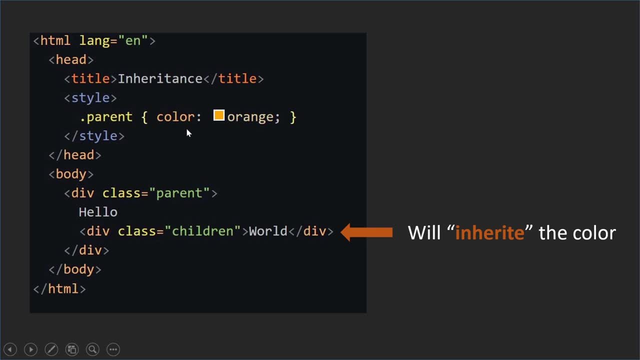 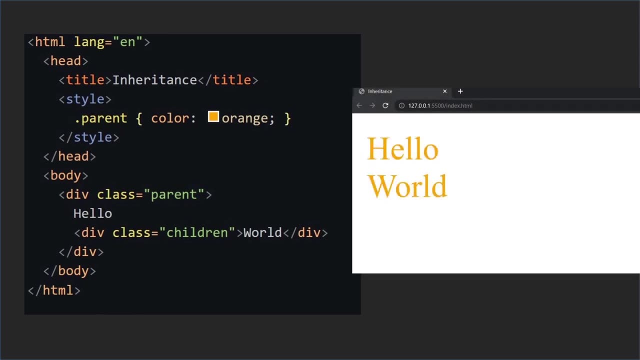 mean by all of them. that's because we are providing a typography style. like color is a typography style, so it will be inherited. just show you the result of this code and this is how it will look like. so now let's just learn about like which kind of things will be inherited and which kind of things will not be inherited in. 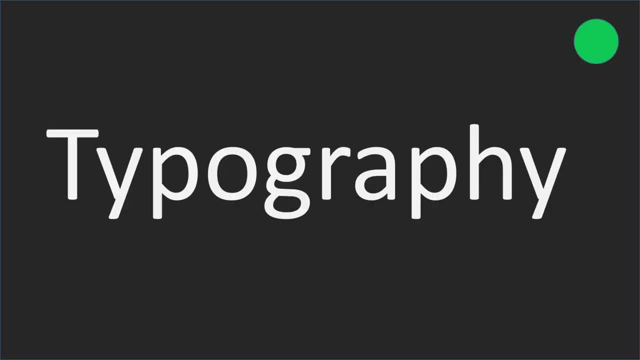 css. so not everything is inherited. so only typography related style will be inherited, and other than that nothing will be inherited. so if you want to force inherit there, so for that you are going to be using something called inherit keyword. okay, so only typography related topics or style will be inherited. so here you can see that group. 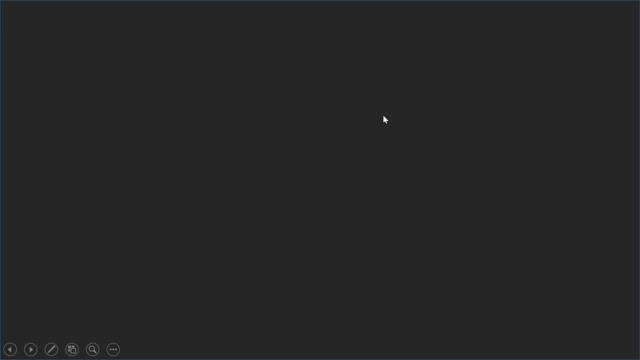 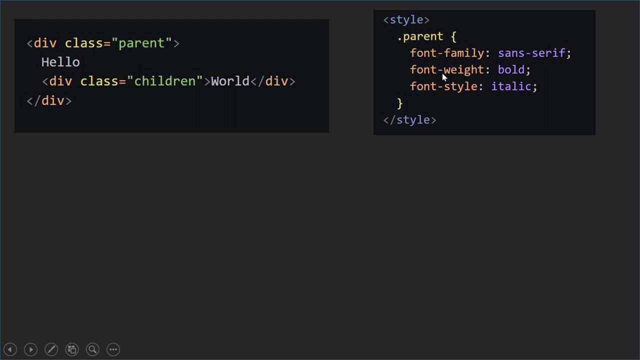 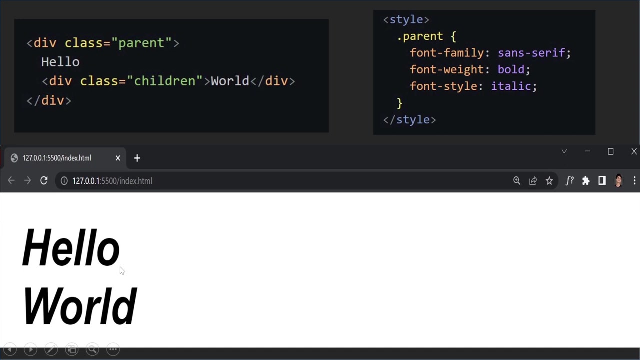 and css will be Declaration hallmark of class. so for example, Now let me just show you a few codes, so here you can see we have a parent and then we have a children and we have the css- like we have a foreign family- of sensor of phone, red of board and font style of italic, and these three can be counted as a typography related styles. 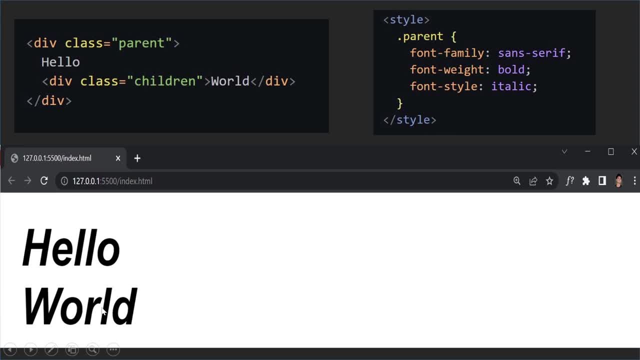 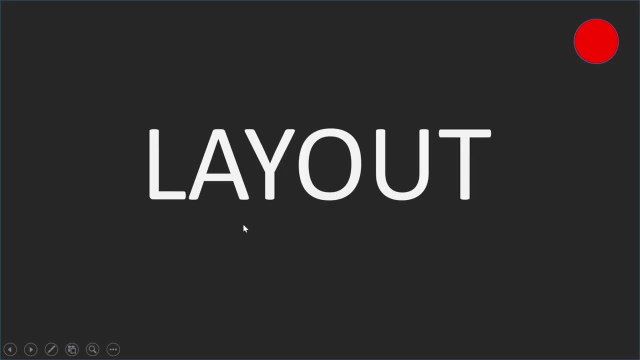 right here inside a children as well. this is a parent one and this is a children one, so both will be inherited. on the other hand, layout cannot be inherited, so all of the stuff which is layout related will not be inherited as a children. so what do i mean by layout, a layout we just discuss? 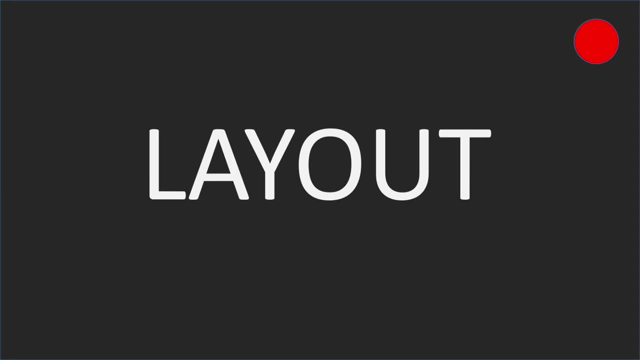 a little bit about layout, but we are going to be discussing more about layout, like we are going to be discussing position, and we are going to be also discussing about display property, like display flanks and css grids and stuff, but all of them will not be affected and now that we know just 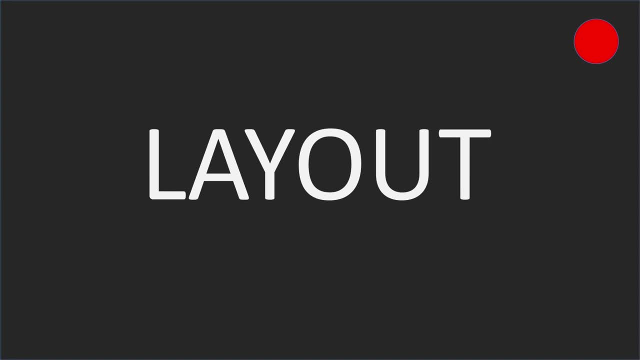 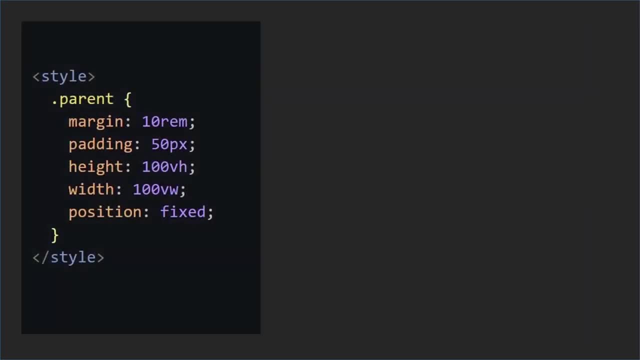 about width and height, margin padding and all of these kind of stuff. so they will not be inherited. so what do i mean by that? so now let me just give you a quick example of that as well. so first of all, we just have this code, so we have a margin padding and height and width and position and all. 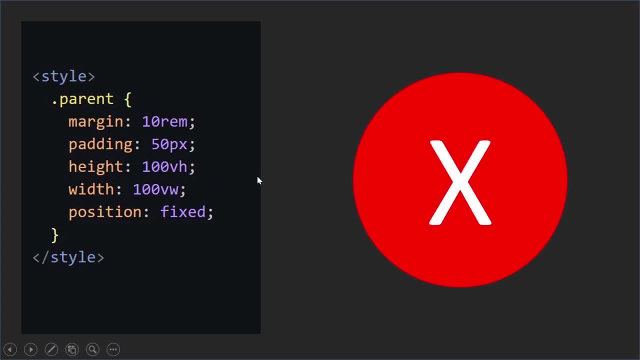 of them are inside a layout category, so these will not be inherited. so i want you to just keep these few slides in mind, and now let's jump into our quarter and write some code, and then you will get to know what i'm talking about. all right, so we are back inside our body tag and now here, what i'm going to do is that. 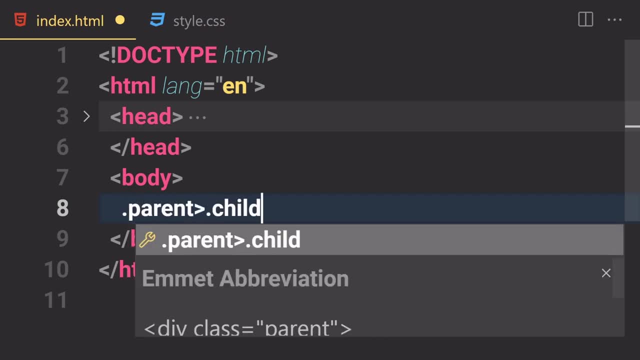 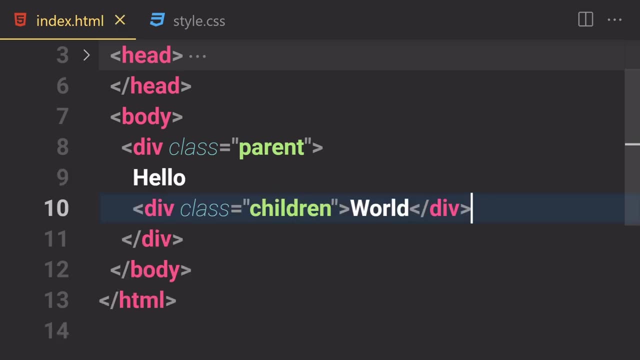 first of all, i'm going to write like a parent and then inside this parent, i'm going to just write our children. okay, so here i'm going to just write like hello, and inside this div we are going to be writing our world. and now, if we save that, so we have a parent with the text of hello, we have a. 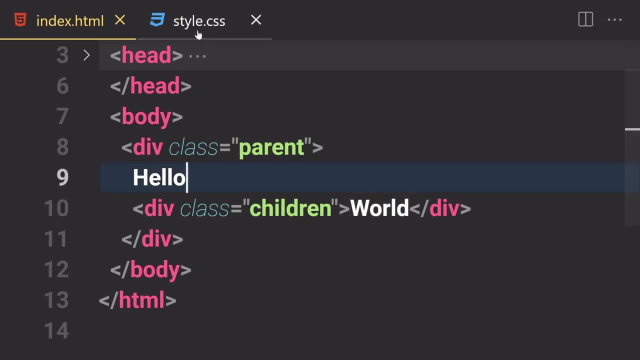 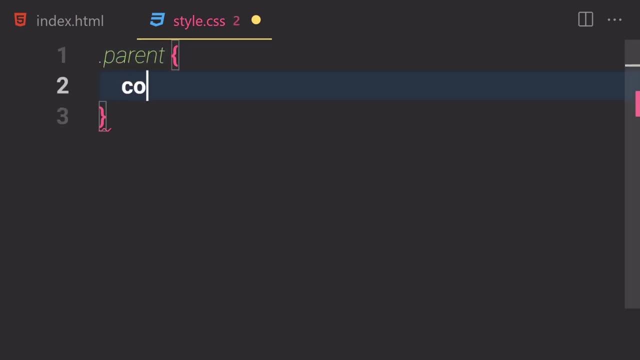 children with the text of world. and now what we have to do? we have to just go to our css and first of all, let me just select my parent, okay. and now let me just provide a color of um, maybe orange, and let me just provide a font: family. 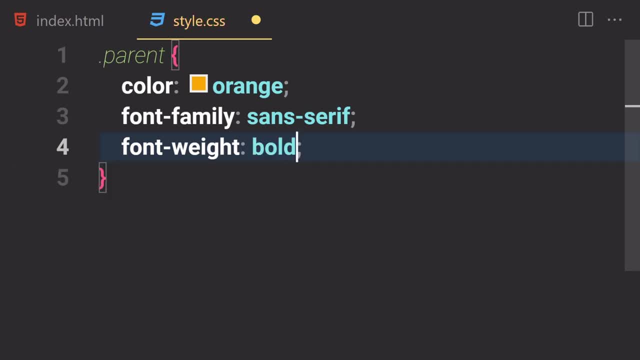 of sans serif. let me also write a font weight of bold and let me also write a font uh size to be like two ram. and i know we have other like typography styles, but for this case we are going to be just sticking into just a few of them. so now i'm going to just save my file and here you can. 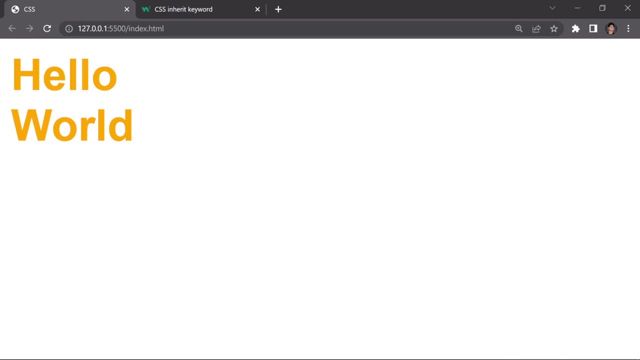 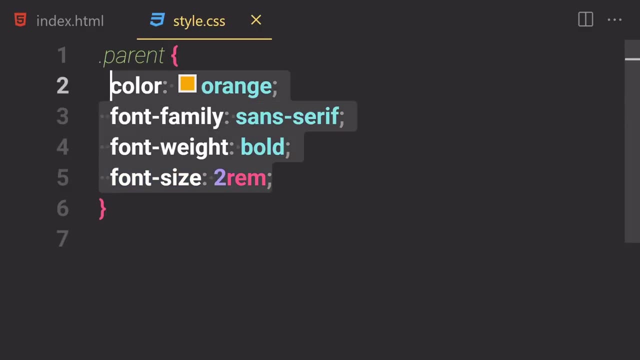 see, the font weight is changed, the font style is also changed and also the color is changed. so both of these will be affected as the way we expand word because we are working on a font property or typography related properties. so these will be affected on the children right here, okay, but on. 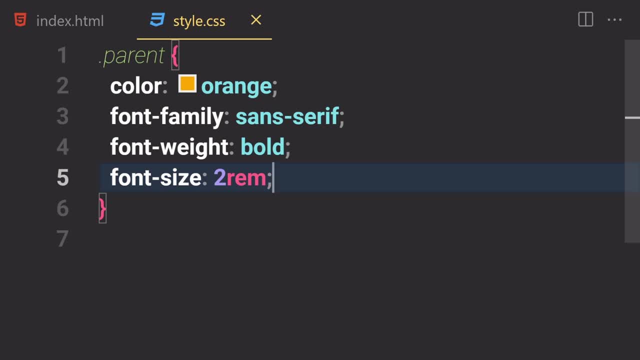 the other hand, if you just write like: uh, first of all, you know what? uh, i'm going to just do a bit of magic right here. you don't have to worry about this score from now, but what i'll do? i'll just select my children right here and i'm going to just provide a position of: uh, what i'm going to. 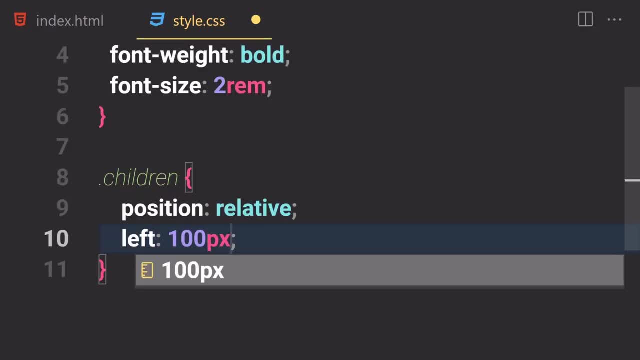 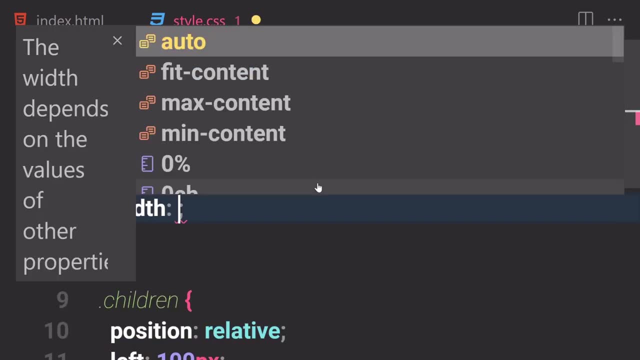 provide a position of relative and i'm going to push there to like 100 pixel to the left and i will save that and we are going to be just pushing that right here and now. here, what i'm going to do is that i'm going to just provide a width of like 100 pixel and i'm going to also provide a height. 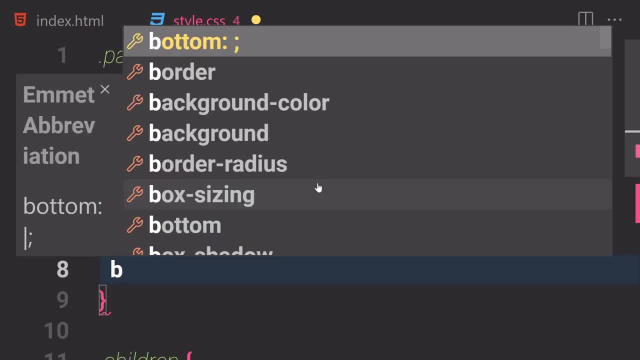 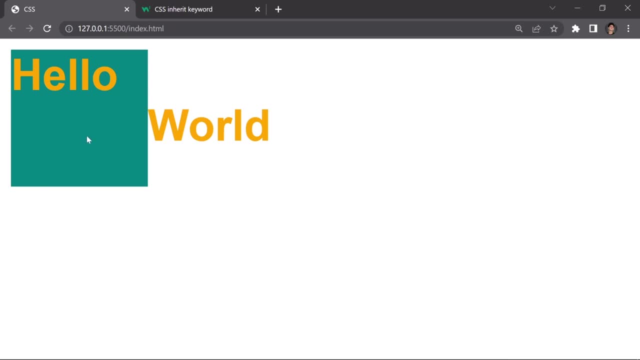 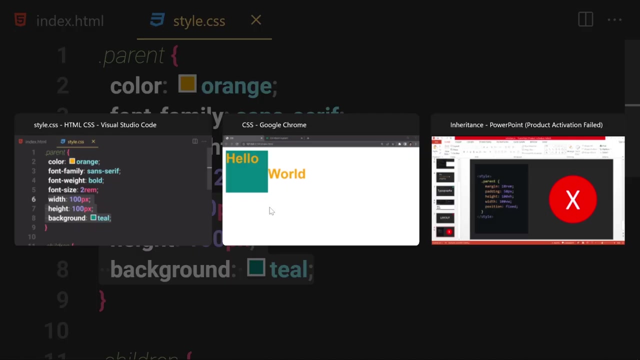 of also 100 pixel, and now i'm going to just provide a background color to it and it will be like a teal kind of color. and now, if you save that, so here you can see, these are now applied to only this one. why is that? because all of this property will be count as our layout property, so that's why it cannot be. 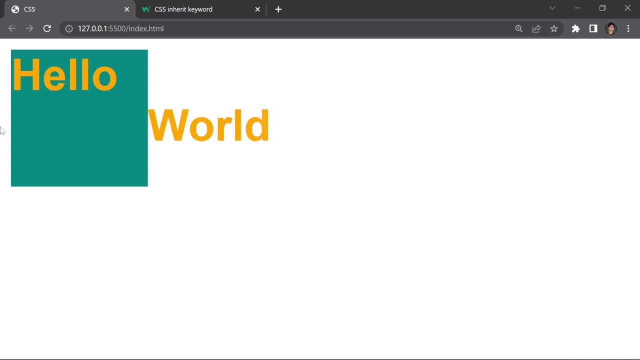 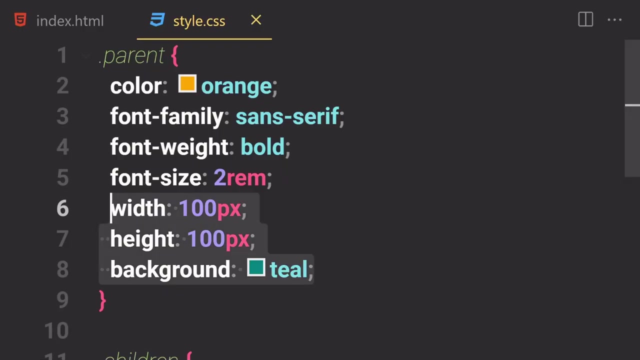 okay, so here you can see. we have like width of 100 pixel- uh, not 100, yeah, 100 pixel- and also height of 100 pixel, and also the background color is also changed, but it will not affect this one. this one is still our children right here, but this one will not be affected because, um, we are working on layout. 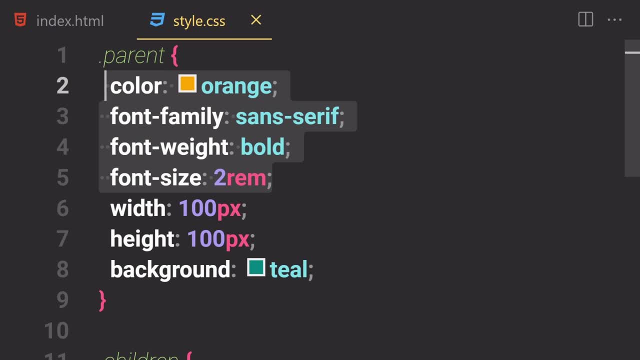 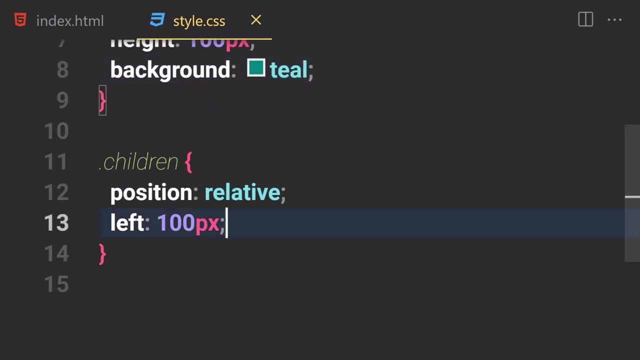 properties. the font related property will be inherited, like a topography property will be inherited, but not a layout one. okay, so you just have to keep that in mind and you don't have to worry about this position relative, and you don't have to worry about this position relative and 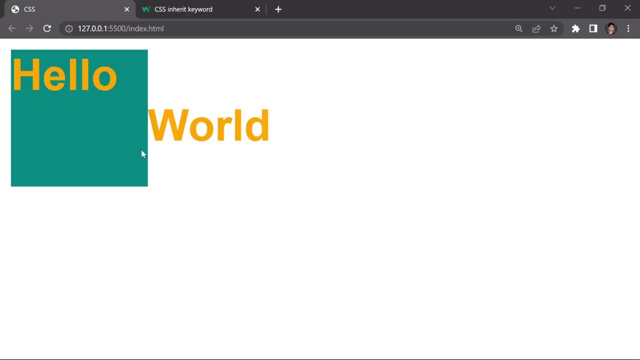 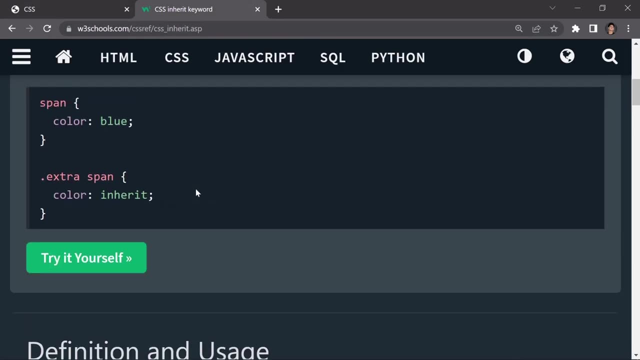 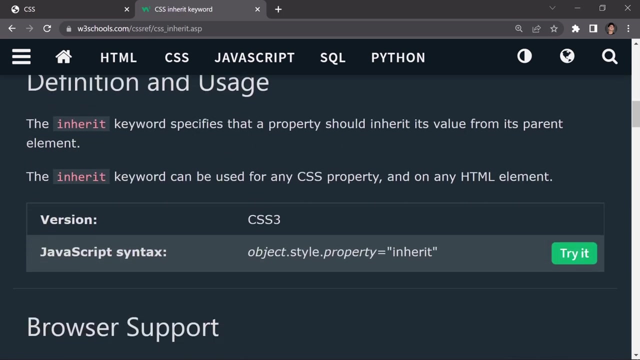 left and stuff like that. now, if you want to inherit this property as well, like if you want to also inherit this width and height properties, so for that we have to go to our mdn or not mdn- in this case it's a w3 school- and now if you just scroll down so we have a keyword called inherit, so let's. 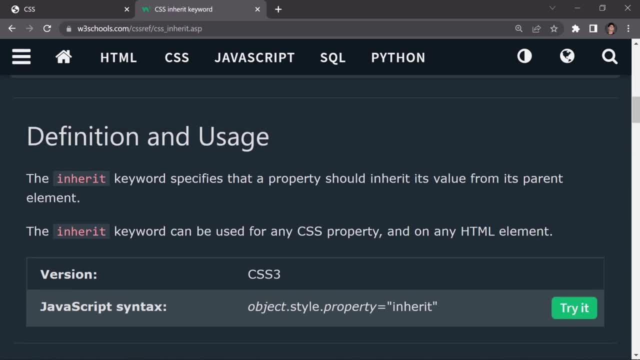 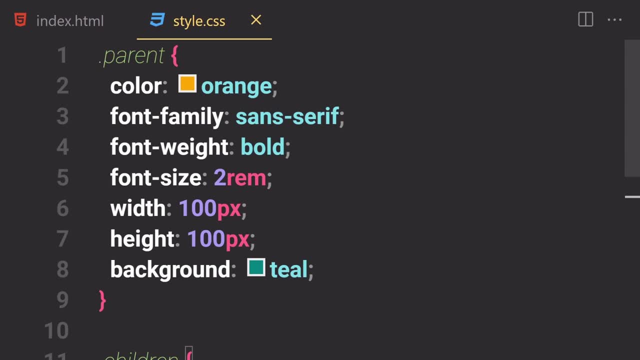 just talk about its definition. the inherent keyword specify that a property should be inherited its value from its parent element. okay, so it will now force all of these values, like we have width, height and back. so now we have a key word called inherit and we have a key word called 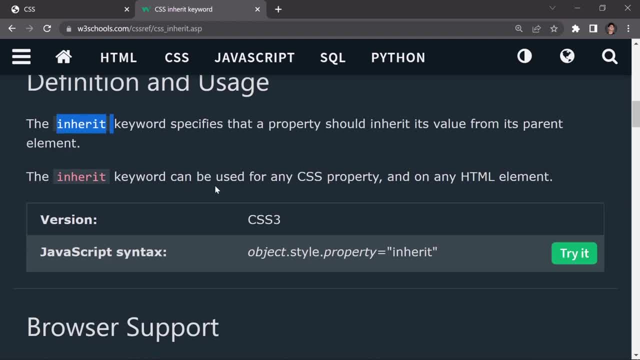 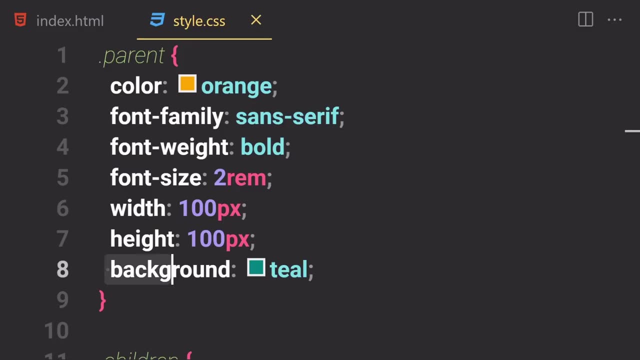 background color to be inherited as a children. so the inherit keyword can be used for any css property and on any html element. so this property can be useful in some situation, but it's very dangerous and my recommendation will be to use it just for a typography stuff and other than that i will not. 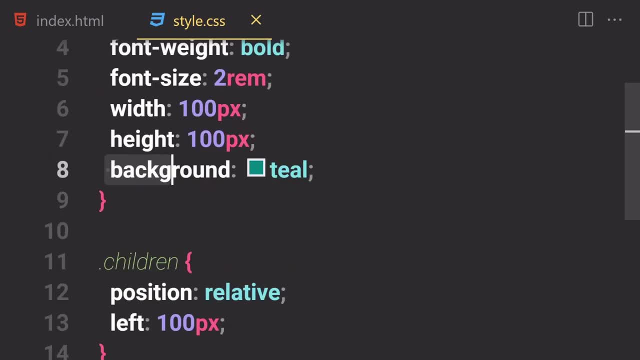 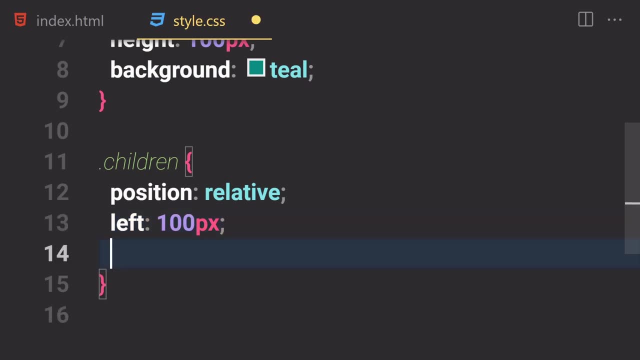 recommend you to do that anyway. so now, if you want to inherit, maybe like um, background color in this case, what do we have to do? so now, we are now inside working on children, so what do we have to do? i'm going to just write a background color and i'm going to remove that color, and here i'm going. 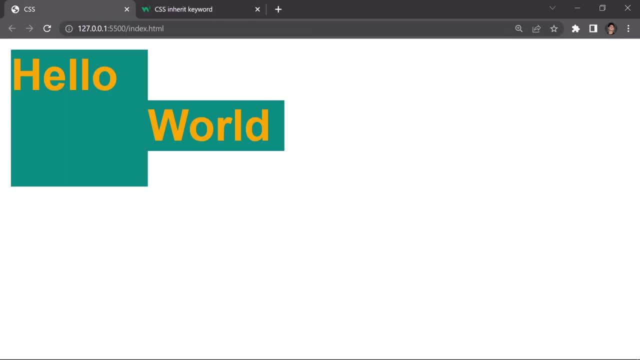 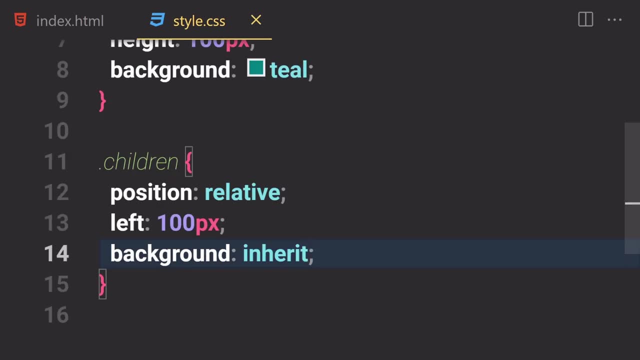 to just write inherit. and now, if we save that, and now if we check and boom here you can see both of them will have this kind of a teal color, right here and now, if you want to inherit this width and height as well. so what do we have to do? we are going to be just writing a width of inherit. 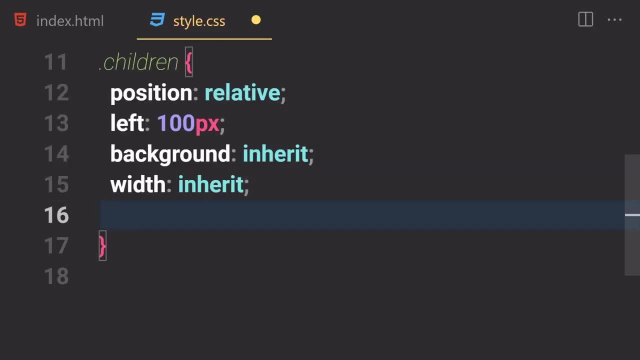 and we are going to be also providing- let's suppose i'm gonna. so, first of all, let me show you the width one, and now, if you save that so here you can see, it will now provide this width to it. but now, if you want to inherit the height as well. so what do we have to do? 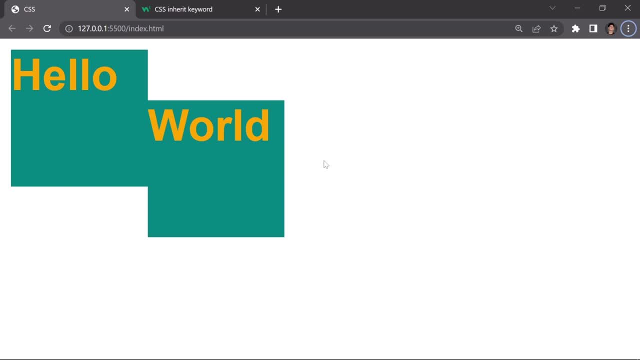 you can just write a background color and i'm going to remove that color and here i'm going to. we are going to be just writing like height of inherit, and now, if you save that and boom, both of them are now looking the same. okay, so now let's suppose i want to increase that to like 200. 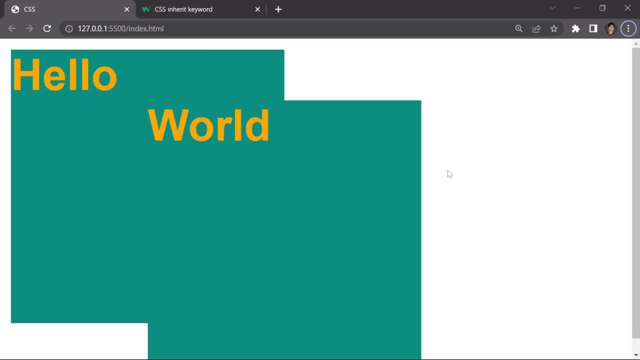 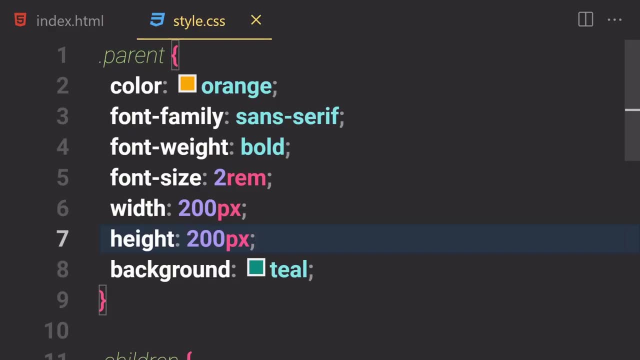 and also this one to 200 as well, and now, if you save that and now here you can see, both of them are now bigger. okay, so this is how you can use the inherit keyword and all of that inheritance work. okay, but in my opinion, i will never recommend you to use inherit keyword. it's kind of like a 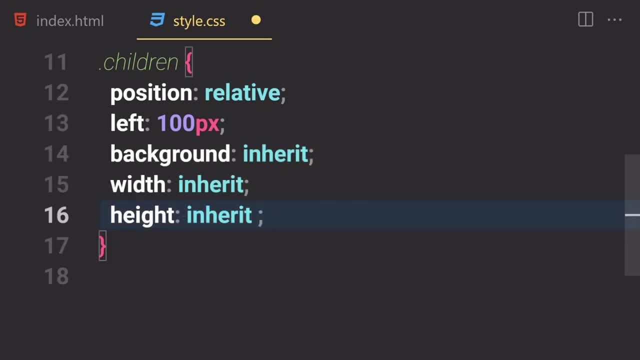 using important keyword which i've never used in my life, have to say, in my life i did use that in some project, but i will never use that, to be honest. so my recommendation is to not use that. other than that, it's all dependent on you if you want to use. 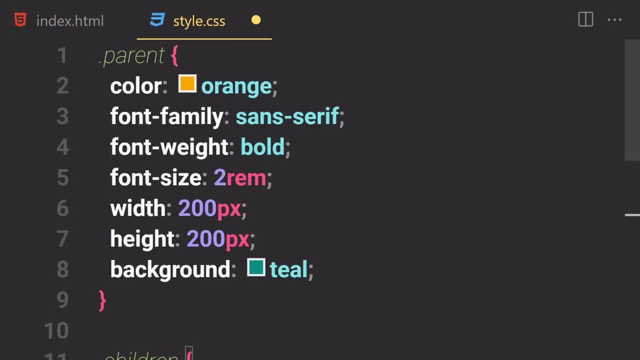 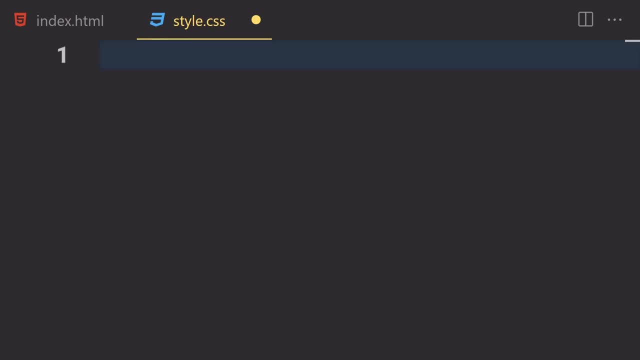 that, so you can use that. if you don't want to use that, so you don't have to use that. i just kind of want to show you, like, what is the inheritance in css. so for now, we are going to be removing everything we have and, boom, everything is gone. so i'm going to also remove these parent and. 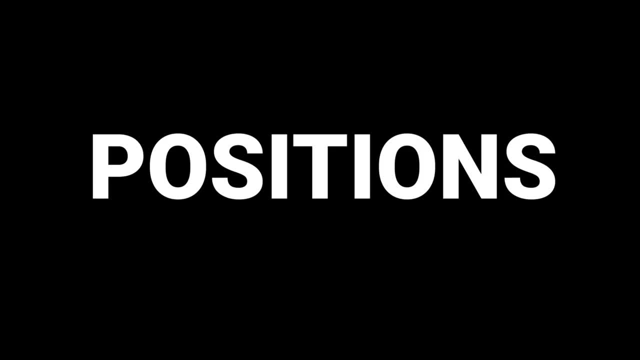 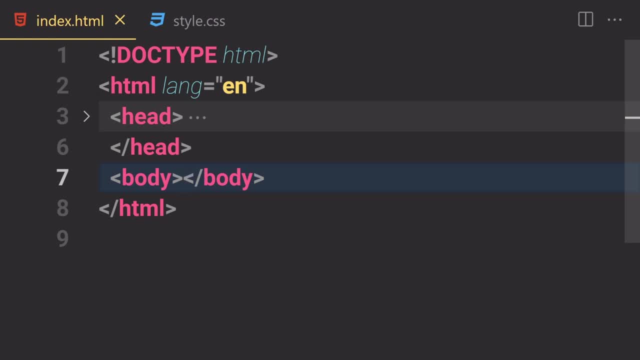 children as well. so save it and we have a clear body alright. so now that we learned enough about a css inheritance, now the next topic which you are going to be learning will be included as a layout topic. so in layout we have like a few topics which you 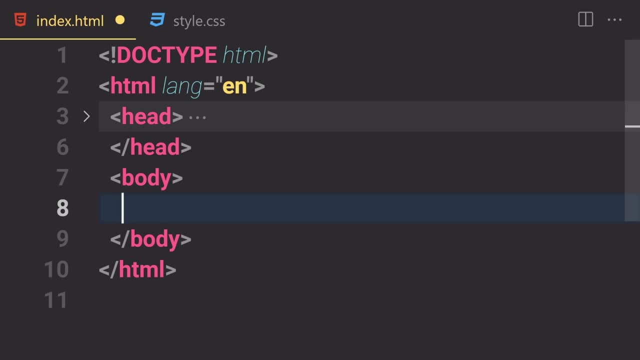 are going to be learning like? first of all, we are going to be learning about position. second, we are going to be learning about flex. third one, we are going to be learning about grid. so, before getting into that advanced topic, first of all let's just start working on our position: property. so we are 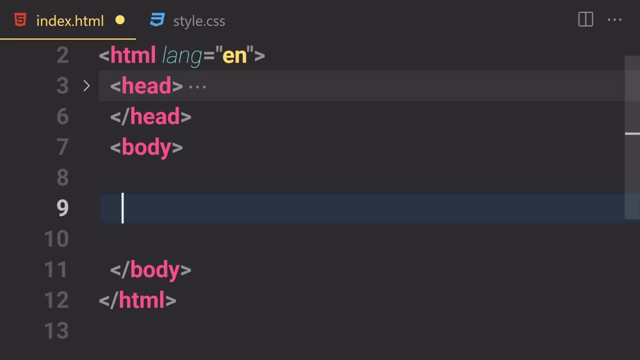 going to be jumping into the position property, but before we do, i just kind of want to say that we have to give a little bit of attention to that, because this can be a little bit tricky to learn. so we are going to be starting from. first of all, let's just create a container inside this container. 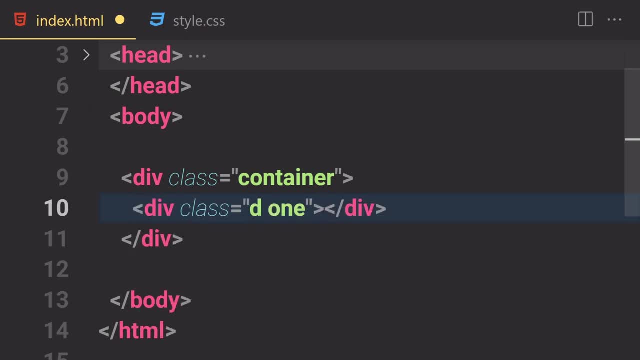 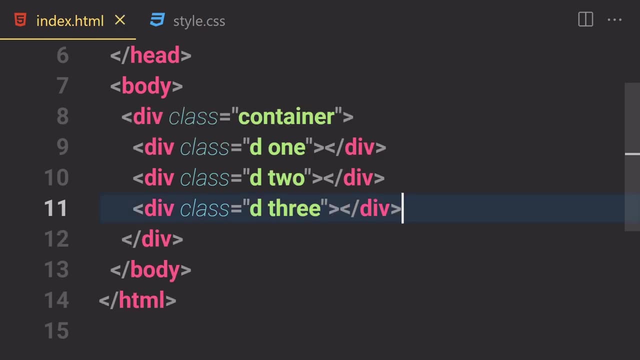 we are going to be writing like two classes, like d and one. okay, so i'm going to duplicate that three times, and then now let's just change that to two and this one to three, and now, if we save that, so we don't have any crazy stuff. but we have first of all a div with a class of container. then we provide: 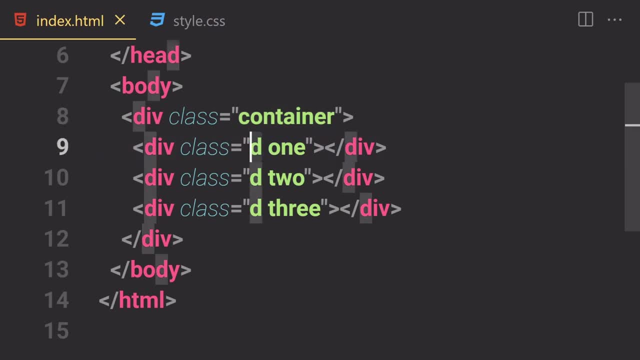 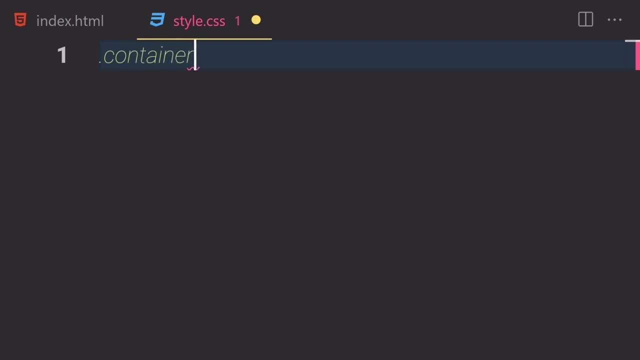 this d class to all of these three divs and then we provide a specific classes, like we have one, two and three. now let's jump into our css and now let's just start styling or div. so i'm going to just select my container right here and inside this container what i'll? 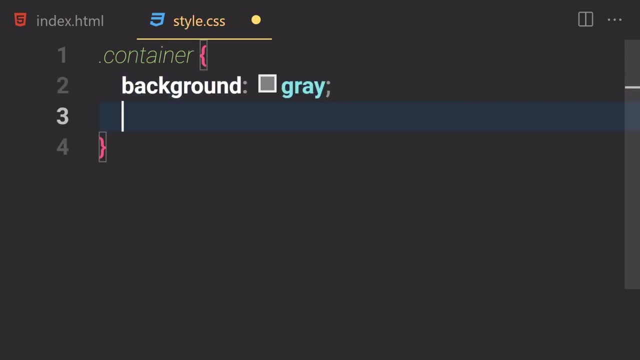 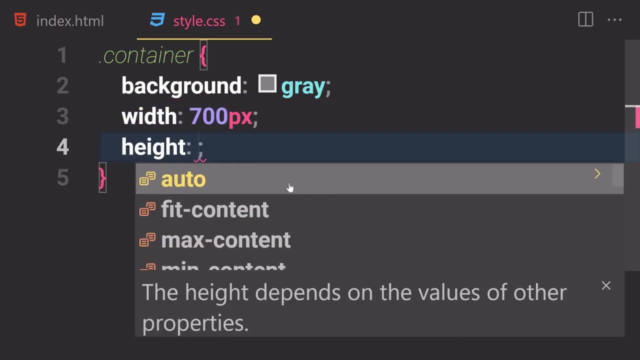 do. i'll just provide a bg of totally gray color and you can choose whichever kind of color you like, and i'm going to provide a width of like 800 pixel or 700 would do the thing- and i'm going to provide a height of like i don't know- 400, 500 would be fine if you save that, so we get this. 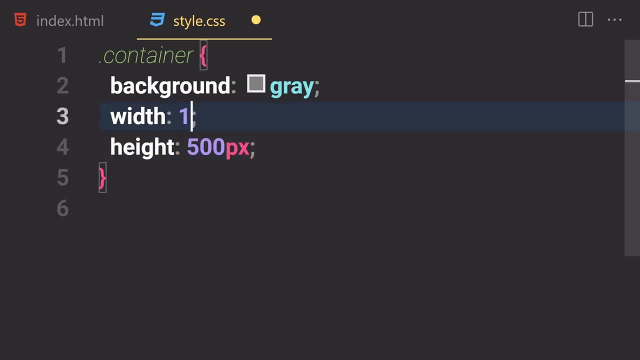 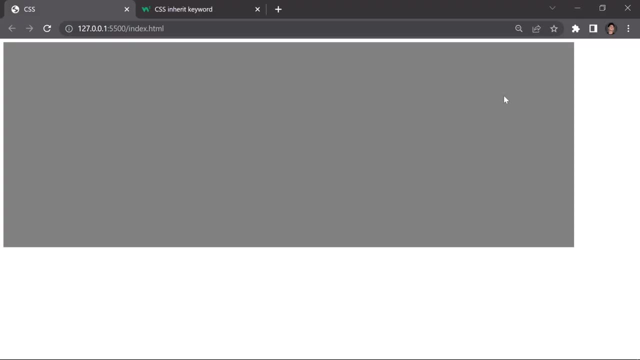 container right here. or you know what i'm going to provide? um 100, save it and this: oh, not 100, just a 90 would be fine, like so, and i guess that's fine anyway. so now we create our first container right here, now, inside that container. what do we have to do? we 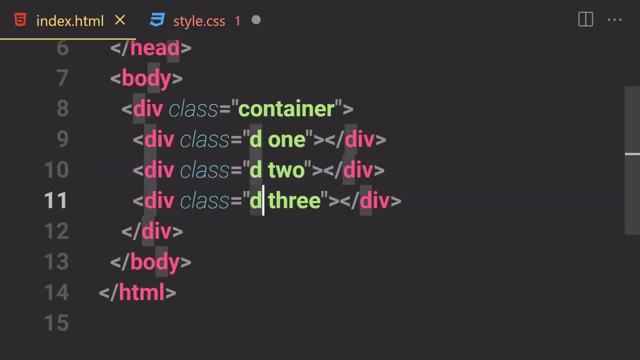 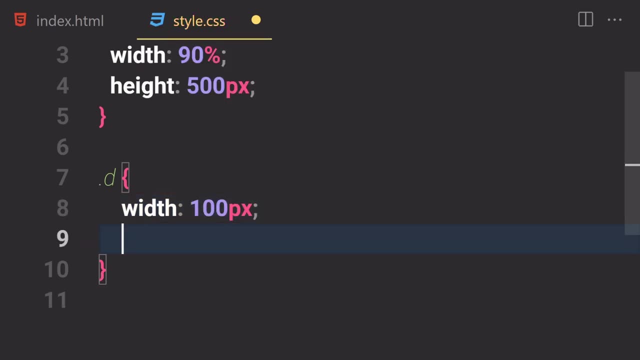 have to select all of the d classes, like this d, this d and also this one, and what we have to do? we have to give them a class of or not class, but a width of like just 100 pixel, and i'm going to also provide a height of 100 pixel. so if we save that, nothing will happen because we didn't select. 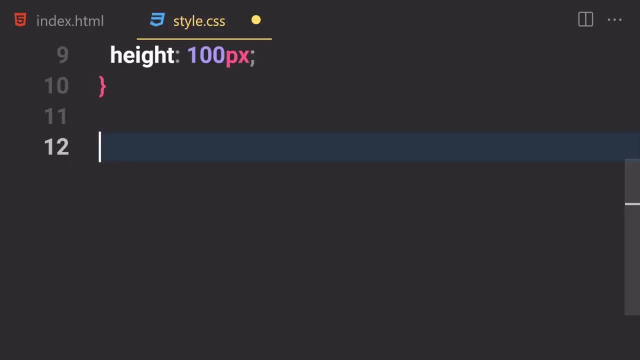 any of these classes and we didn't provide any background colors to it. so now let's just select our first one and provide a background color of red or teal would be fine- uh, not teal. i'm not going to provide any teal, but red will be fine red. and then let me just duplicate it two times. then we have the second. 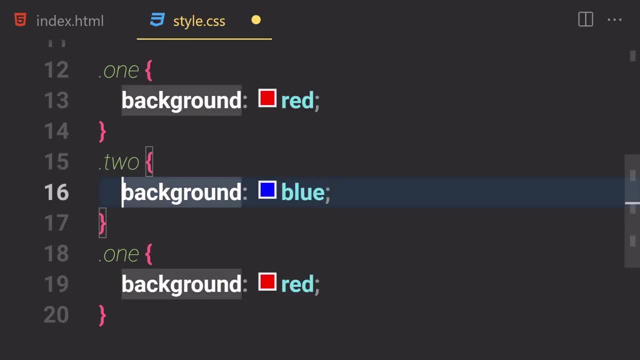 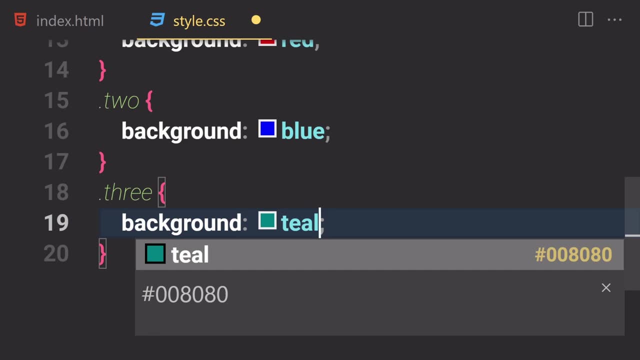 class like two, and here we're going to be providing a blue, and then we have finally the third class, like a three, did we just? yeah, we have three, and this one will be kind of a teal class. so I'm going to just zoom out of it and so that we can see everything a bit better, 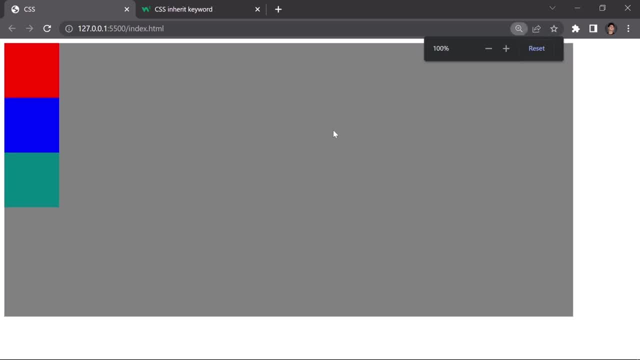 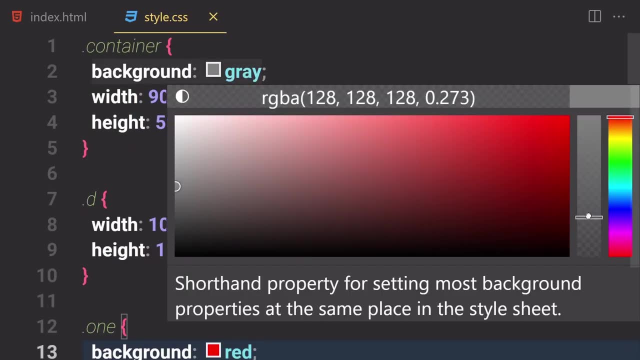 so now, if I save my file now here you can see we have this gray kind of container. inside this container we have these three uh deals right here. so now let me just change the opacity of that. will be like just a little bit slider, not that much. come on, I want to change the color to be like: 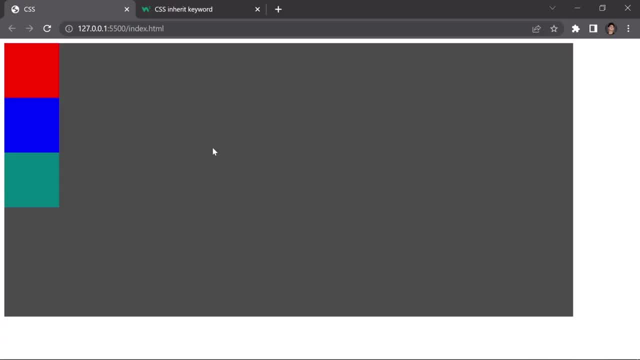 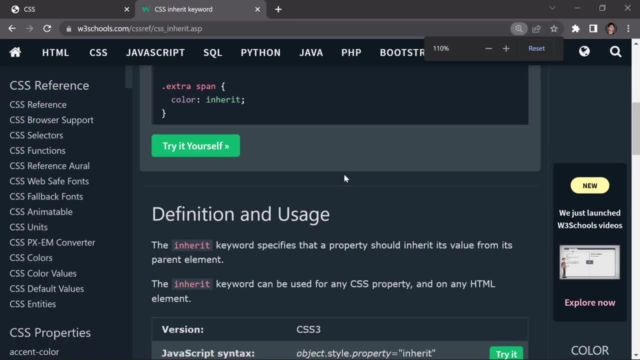 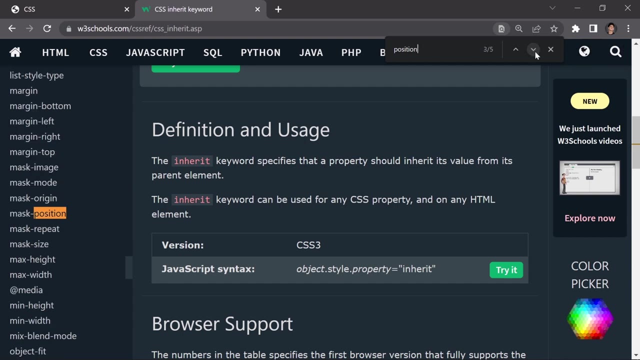 something else. maybe that's that much kind of a grayish seven and yeah, that's looking cool anyway. so first of all let me just show you that relative and stuff properties. so first of all let me just position. okay, so we have background position and we have position style and mask position. come on. 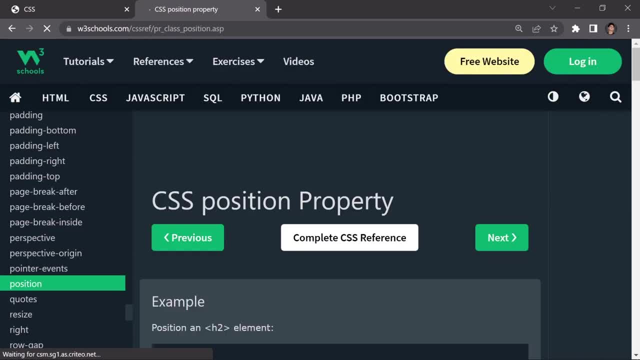 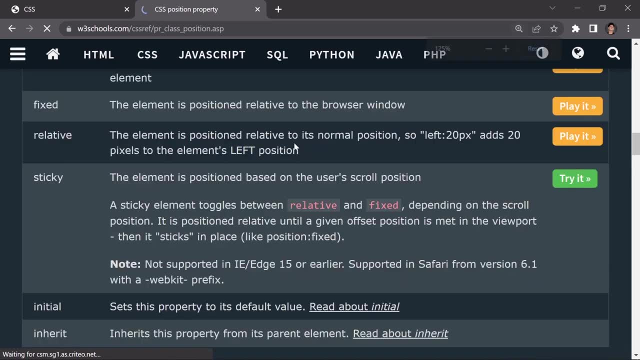 and then, finally, we have this position property. if I click on that, it all brings us to this page right here. so we have position H2 and a lot of stuff and let's just scroll down a bit. so we have a few position properties. so the first position property which we are going to be using- uh, I mean, 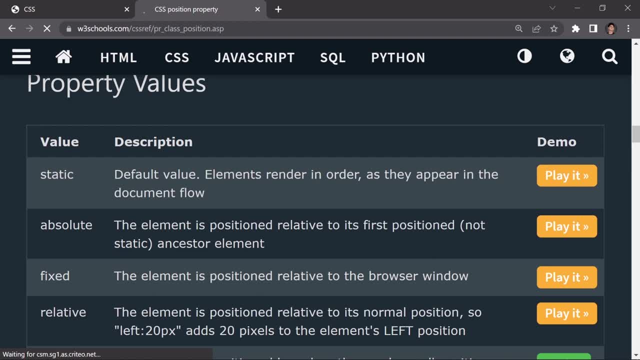 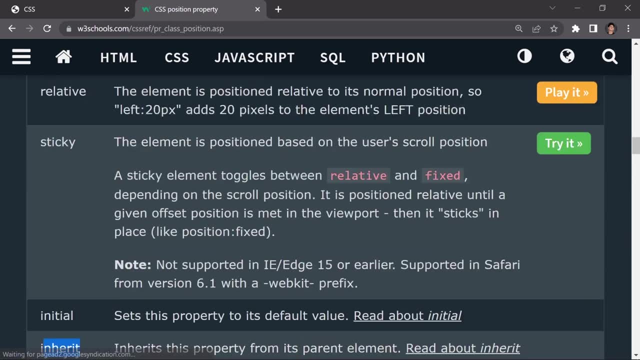 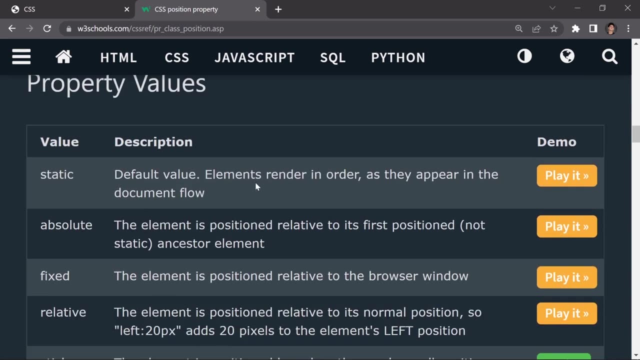 like. we have a few position values to be precise, not properties. so we have a static one, we have absolute, we have fakes, we have relative and we have sticky. okay, and these are initial and inherit. you don't have to worry about that. we already learned about inherit in a previous section, so static will be the default value, like by default elements. 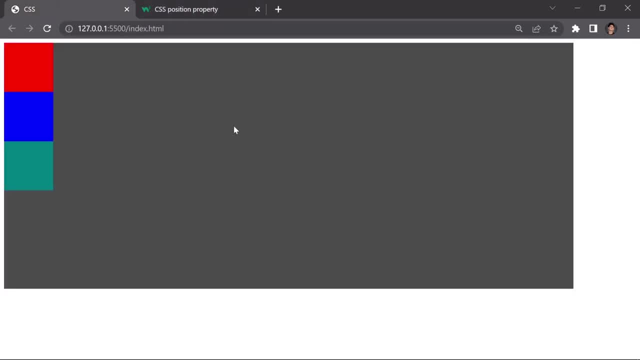 render in order as they appear in the document flow. so if you check there, so here you can see first of all we have the one, then the second, like a two, and then we have a third one. so these are at the top of each other. so this is known as a position static. okay, and this will be the default. 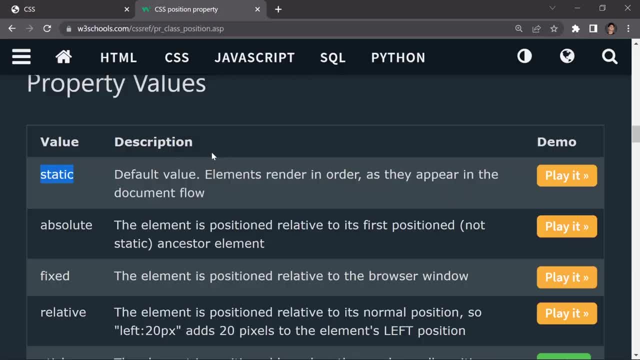 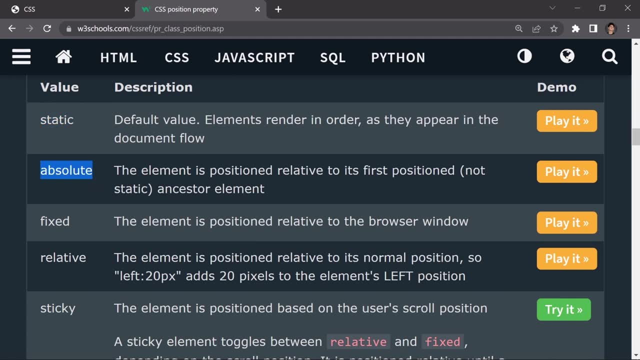 position of, or um, or off our side, okay, or layout, or whatever you want to call it. so then we have absolute. the element is position relative to its first position, not static and sister element, okay. so what do I mean by this gibberish? but before getting into the absolute and fixed and all of that, first of all let me just show you the relative. 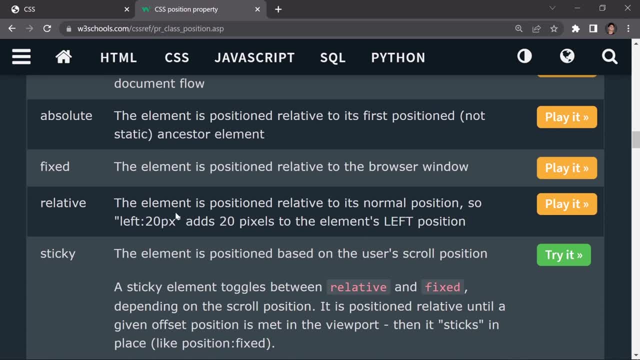 one. so now let me just read it. it's description: so relative, the element is position, relative to its normal position, so left, property. and we have a lot of properties like left, top, bottom, right and these kind of properties which I'm going to show you just in a second. add 20 pixels. 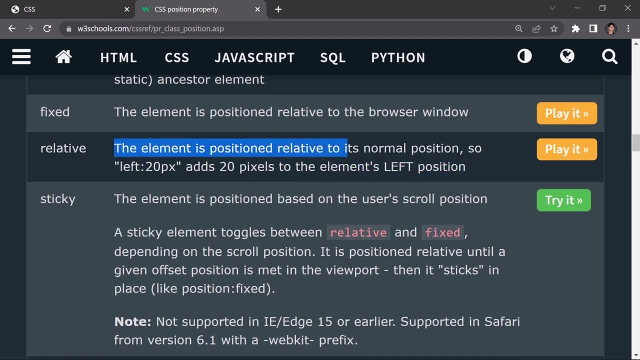 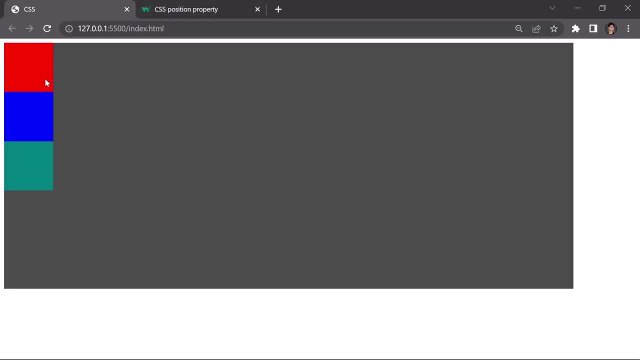 to the elements: left position. okay, so you just have to remember this first line. like the element is positioned relative to its normal position, so by default, if you check over red one, so it's just position normally right here inside this container. so now, if you want to just move there, 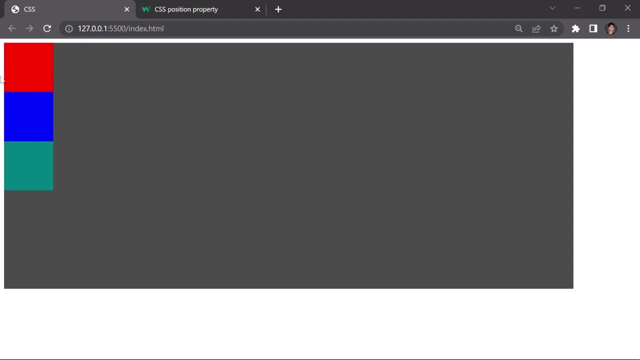 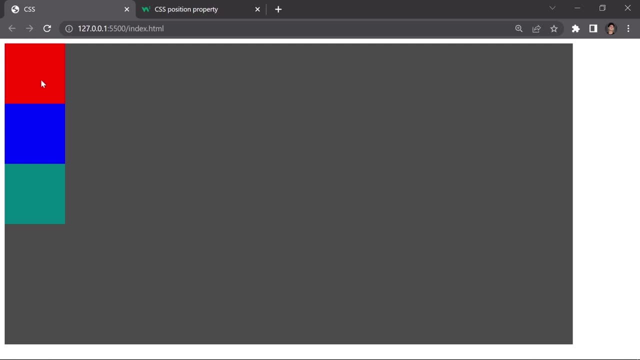 to the left, so we can also move there to the left, to the bottom, to the top or to the right, but it will be moved where we want to move there. but it will not leave its place. so it will take this place and it will be moved to wherever we want. so now let me just show you the 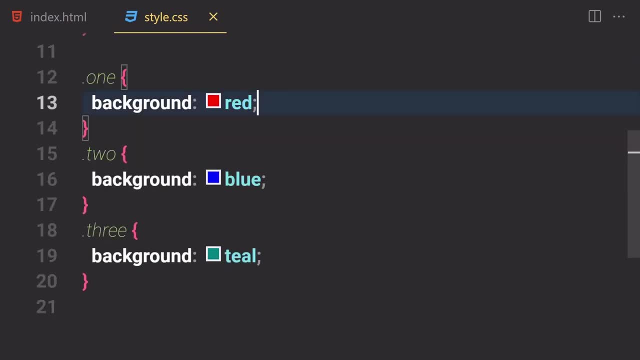 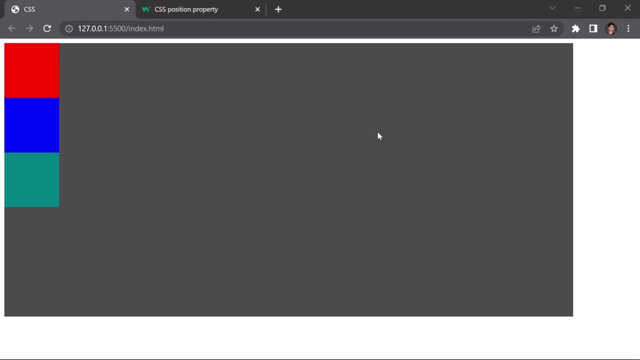 encoding. so we are going to be first of all selecting our first one, which is the red one. so what do we have to do? we have to just provide a position of relative to it. so if you just provide a position relative and if you save there, nothing will happen. well, because we're going to use this. 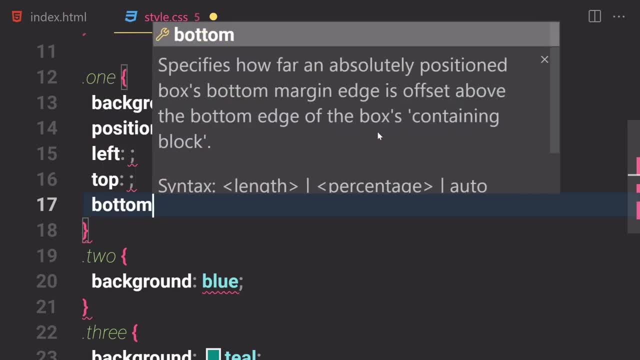 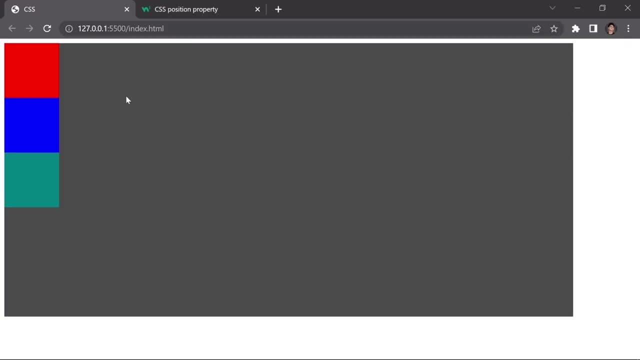 property, like we're going to use left, top, bottom and also the right properties. so now we have to use like any of them. so if you want to use the left one, so if you want to push or container or div to the left, so we can just use left property and then we can specify the. 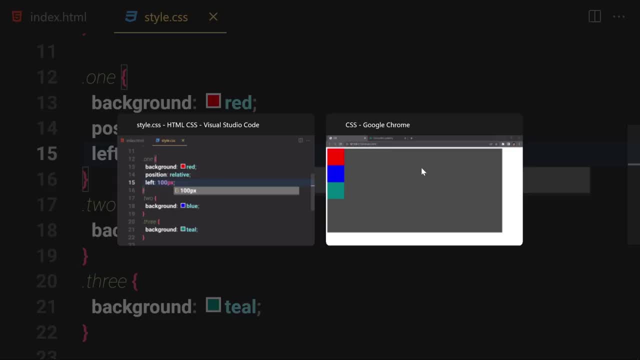 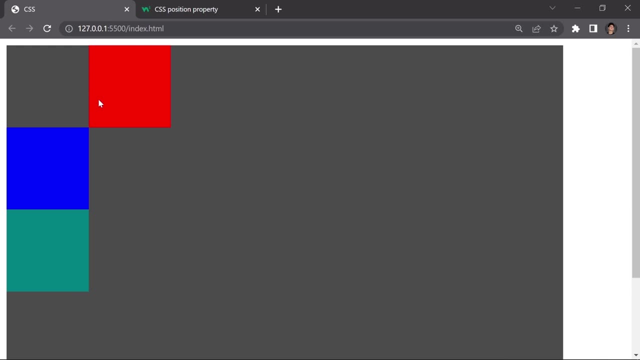 amount like, let's suppose, if we want to push that like 100 pixel and if you save that- so here you can see- it will now push it to the left like 100 pixel, but it will not leave its place right here. so here you can see, we can now like push it to maybe, instead of 100 we can push it to 200, but 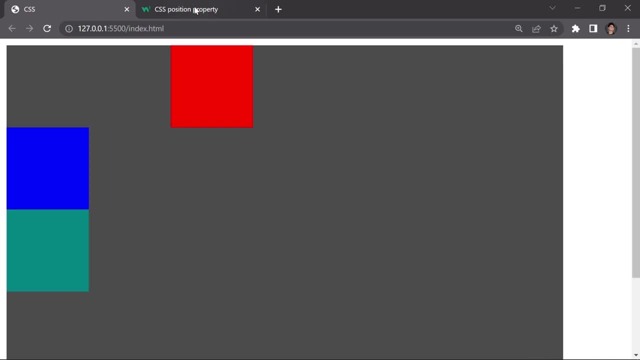 it will not leave its place right here. it will, like, take its place, as they said, like the element is positioned relative to its normal position, but they didn't specify that it will not leave its place. okay, so you just have to remember there for the relative and 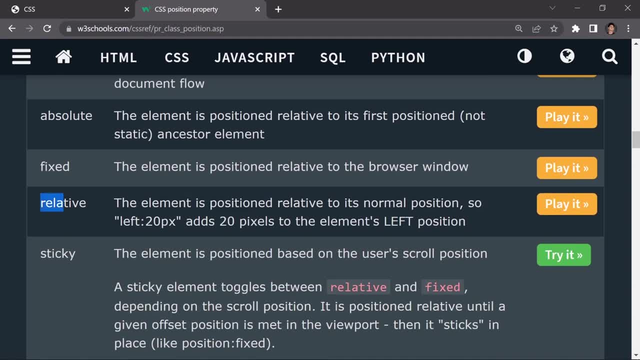 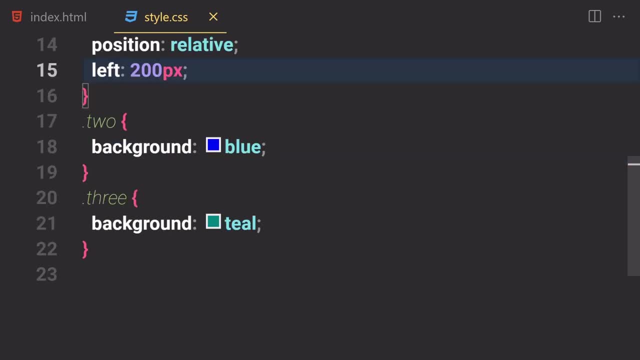 the position. position static will be a default one and position relative will move up to wherever you want, but will not leave its entire space right here. okay, so this is it about a position relative. so now let's learn about position absolute. so the position absolute, the element, is position relative. 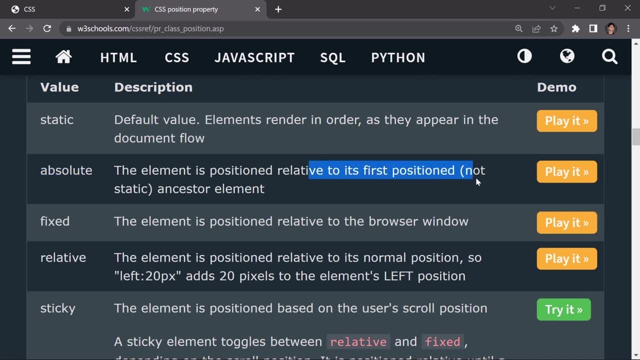 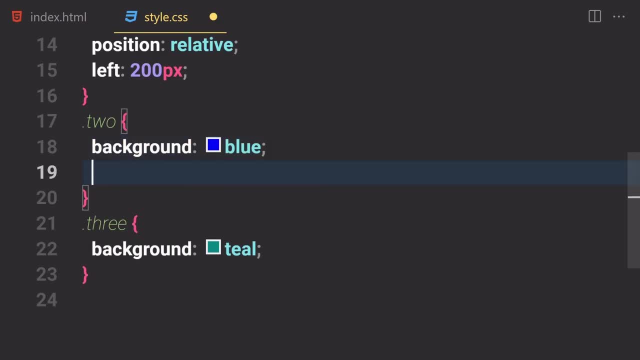 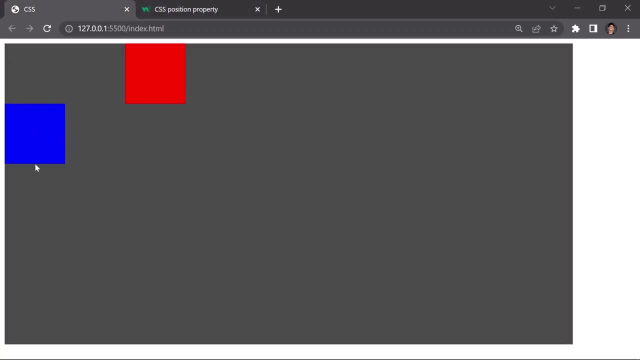 to its first position position, like a first position element, not static and sister element. so what do I mean by that? so if you want to work with the position absolute, so if you just start a position absolute, so let me just start a position absolute in here, and if you save that and here you can see that's gone. so where is the other one? well, because they 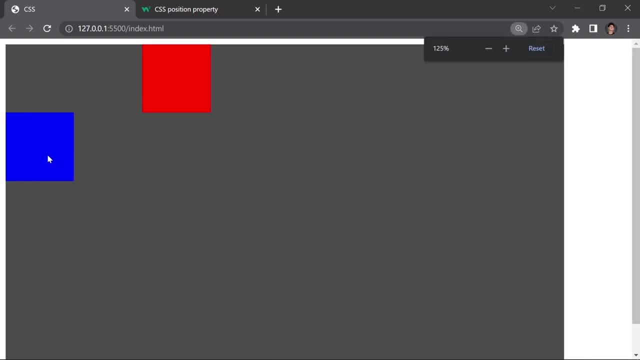 are jammed to each other right here because that we provide a position absolute to it, so it just took its place. position and relative will not leave its place, but, on the other hand, position absolute will leave its place and we can move it to wherever we want. okay, so it will just check for. 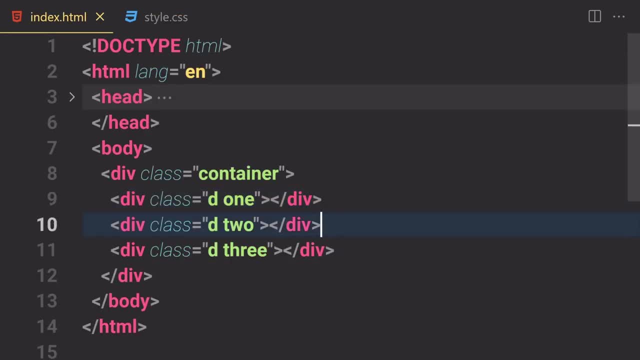 the relative property. first of all, it will just check: uh like, we are now working on a position absolute right here, let me just write it: absolute right here. so first of all we'll check like this: like, do you have a position relative property? yeah, I do have a position relative property, but 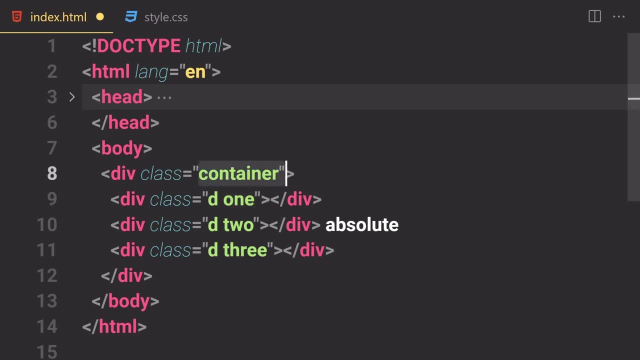 in some cases this will not have a position property. so we'll check it here, like: do you have a position relative property? they will say like no, I don't have, so it will just go to the body and then finally it will go to the element, like HTML root element. so now I'm going to just 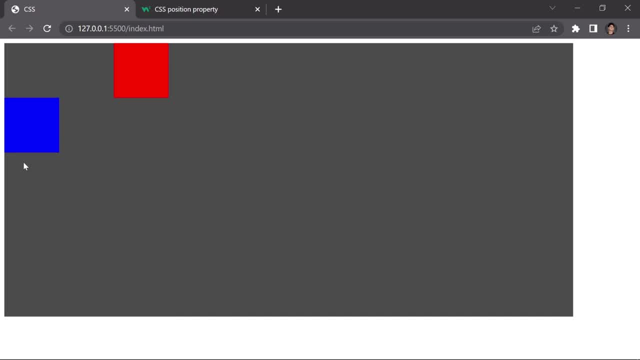 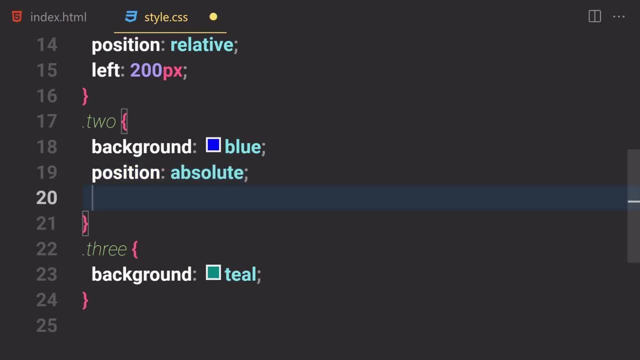 remove this absolute from here and now. if you save that now here, you can see that's gone from here, like the other element is gone. so now if you want to move around there, so for that we can just use our top, bottom and left property. and now if you just write like, uh, left in here. 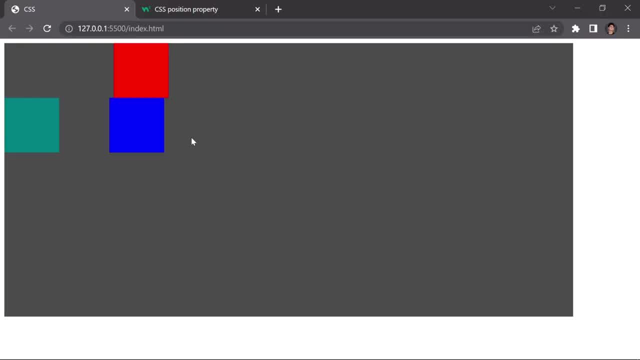 and if you just write like 200 pixel and if you save our file- so here you can see- it will now push it from this area to this area. now, here you can see, this element left its place and we just push that to the right right here, not to the right, but to the left, like 200 pixel. we can also write a top. 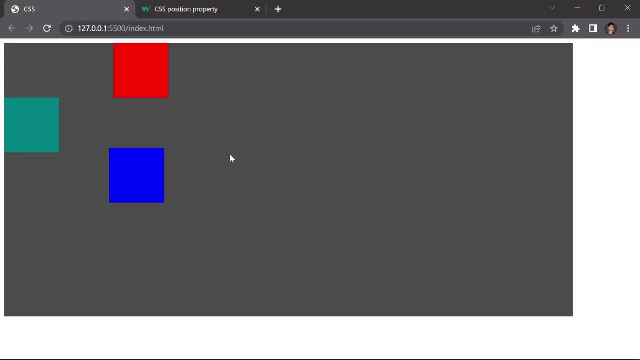 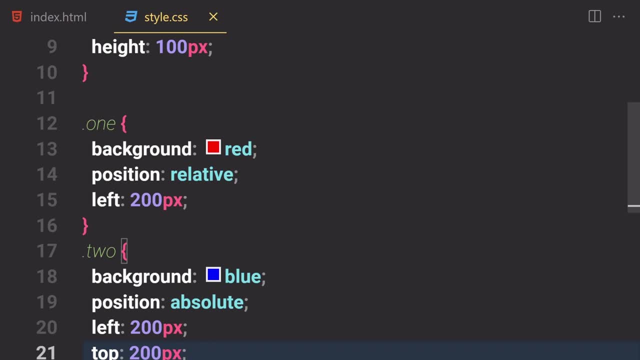 value to it. so top will be like 200 pixel and if you save that, so it will now push it to the top. you can also push it to the right and so on and so forth. okay, so you can play around with that. so we are now totally done with the position static. position relative. 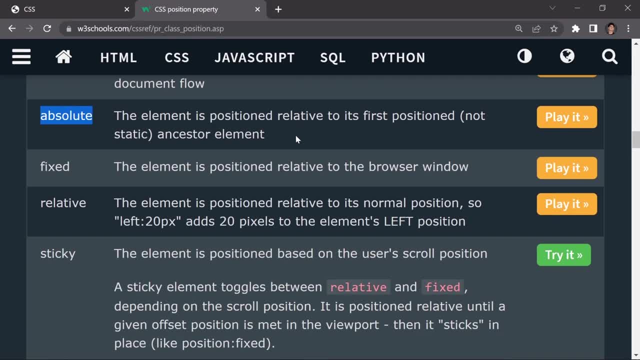 position absolute properties. so now, the next property which I want to talk to you about is a fixed and, as the name suggests that it will be fixed value. so the element is positioned relative to the browser window. it doesn't care about its relative units like, uh, this one on this one, and 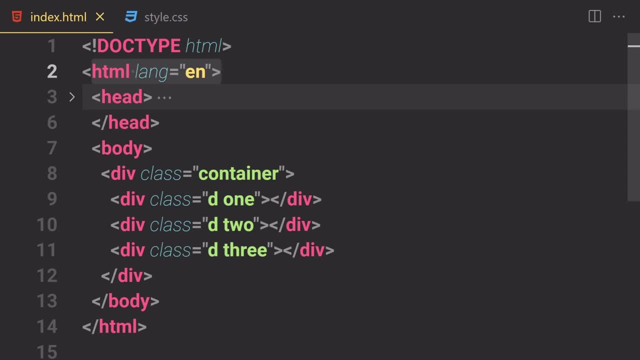 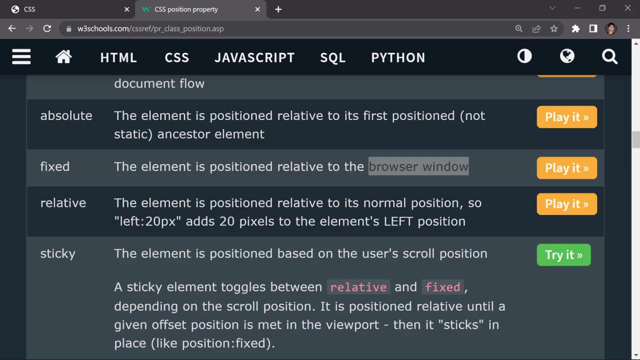 so on and so forth, but it do care about its document element, which is just a root. so if you just write a position fixed to this third one- so I'm going to write a position of fixed to this one- if you save that, and now here you can see, it will be pushed to the top. 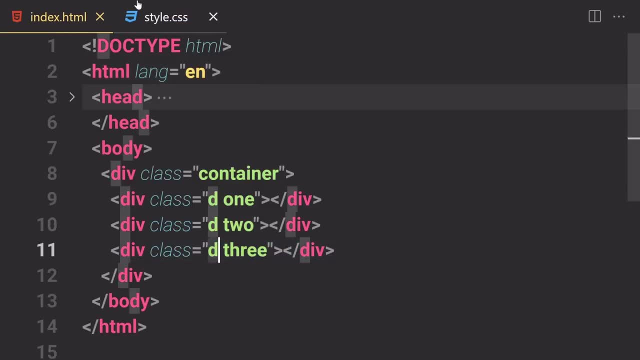 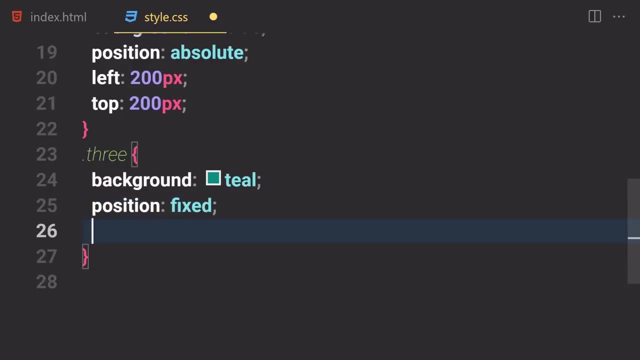 okay, so we cannot provide that. I don't know what's happening. we have THR double E, THR double E, so if you just provide that, so it will now push it to the top. so now let me just write like a top of 200 pixel, and if you save that, so it'll now push it right here. we can also provide it to what we can. 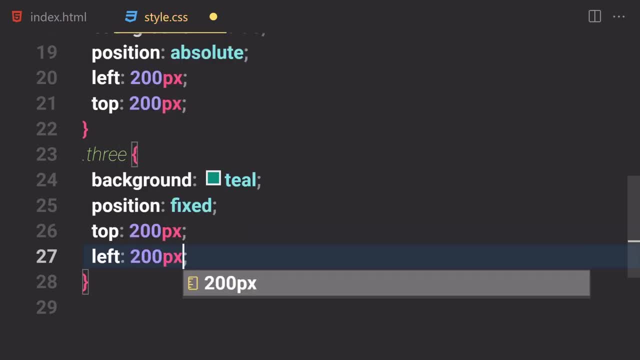 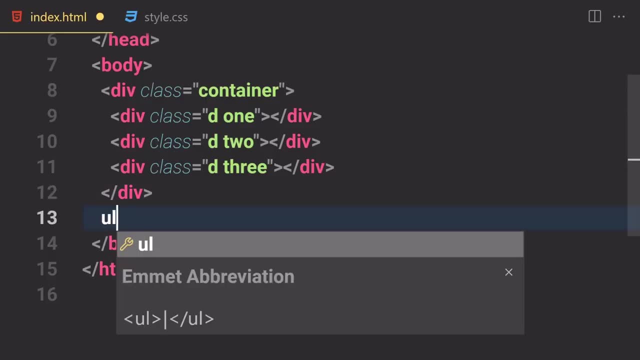 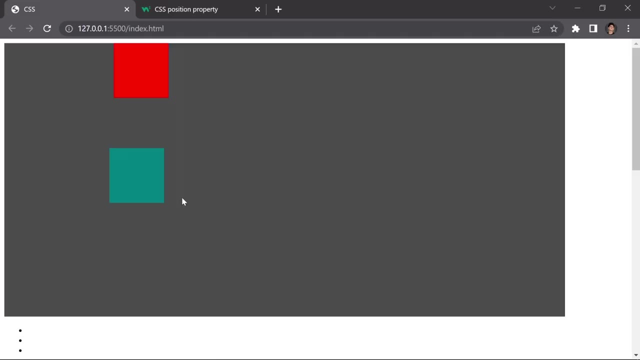 also provide it to like um left of maybe 200 pixel, and now, if you save that, so it will now push it right here and we can also do a scrolling. so now let's suppose if you want scrolling, so we can just do ULLI, and now let's just write like times- uh, I don't know, maybe 50, and if you hit tab and if you 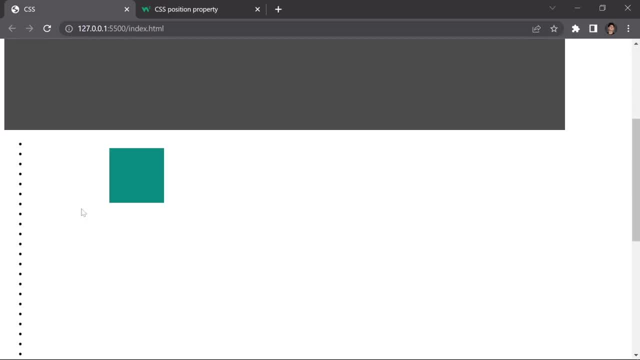 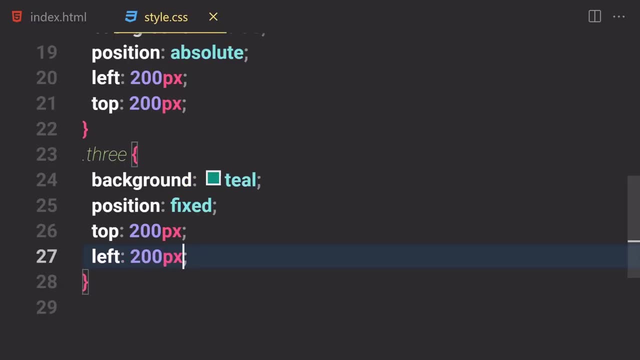 scroll down. so now, here you can see, we have a scroll bar and now if I scroll, so it will just start from this area of the viewport and we can now scroll that to wherever we want. so you know what I'm going to just remove this 200, uh, to the left, or not to the left, but to the top one, so it. 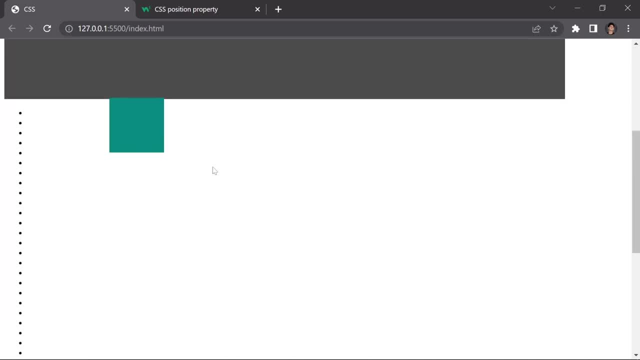 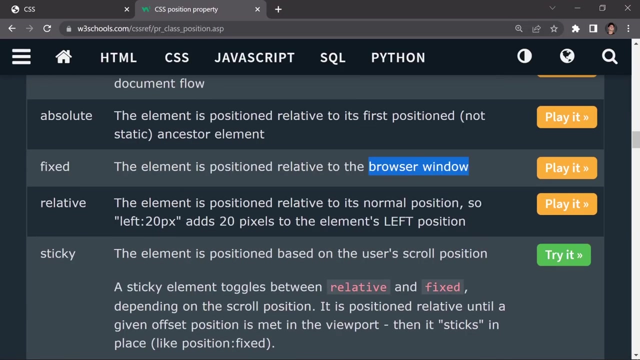 will now be here so we can now scroll over side and this position fixed will be also scroll, and this position fixed property will be very useful for the navigation kind of stuff, so like whenever we scroll, so there will be also the navigation will be also scrolled with us. now the next property we have is a sticky property, which is this sticky: 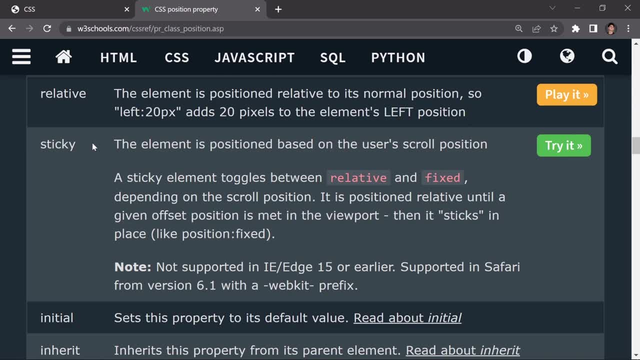 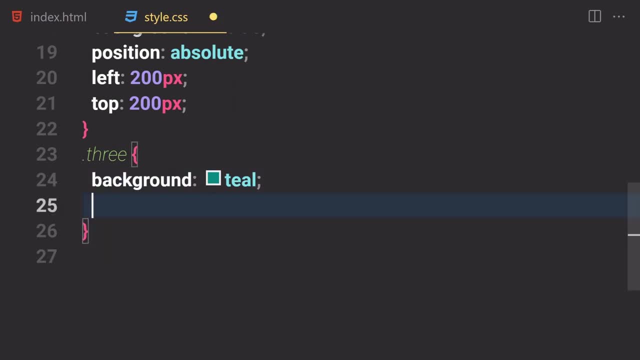 property. the element is position based on the user scroll position. you just have to remember that and it's kind of an easy one. so you know I'm going to remove this position fixed from here. and what do I have to do? I'm going to just provide a position of. let me just write a position of sticky in here. 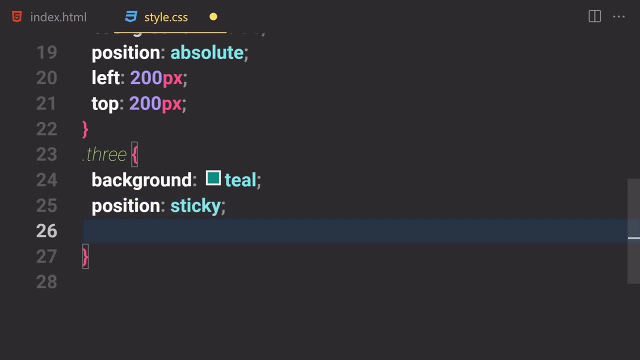 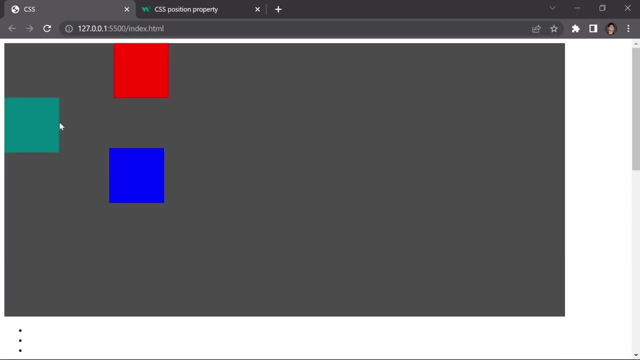 not static but sticky, and now you can just provide some sort of position. like you know, I'm going to provide a top to be like 100 pixel, and now, if you save that now, here you can see it now, push it from the top. and now, if I scroll, 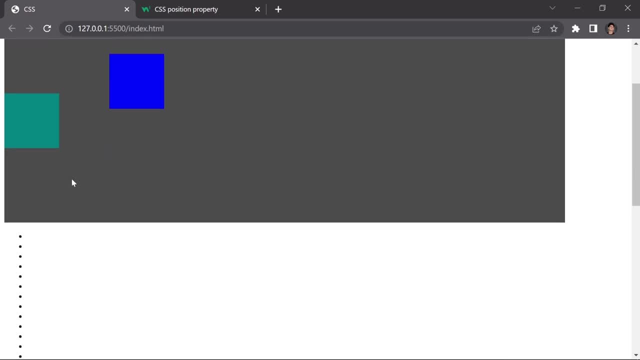 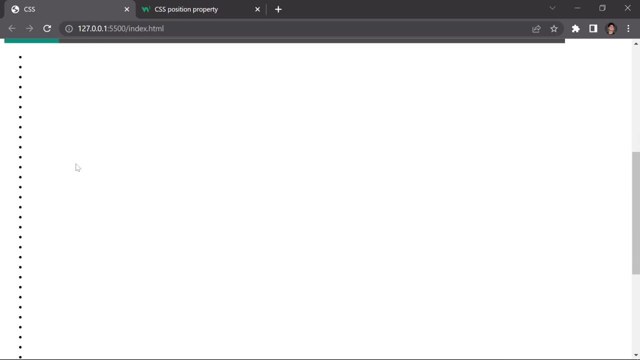 so here you can see, this element will be also scroll, but if we hit this certain point, so that will stop right here, because we are now currently inside this container. okay, we are not outside from it, so we are totally inside this container. so that's why it cannot be pushed down anymore. so 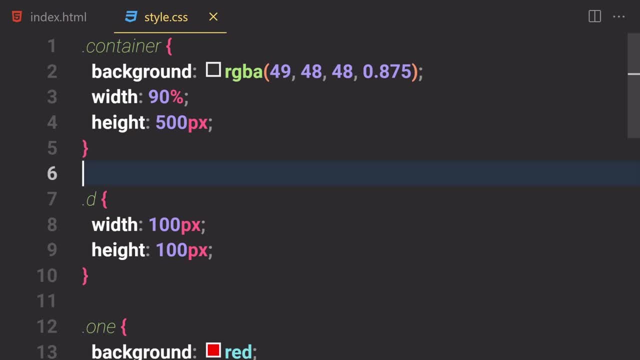 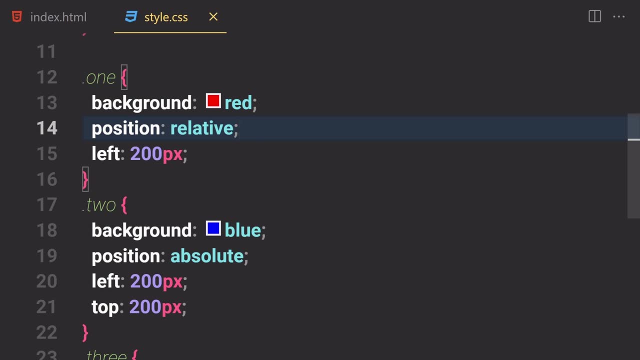 these were just a few properties which I kind of want to show you, so let's go ahead, and let's go ahead and show you. so now let me just review all of them one by one. first of all, we just learned about position relative property, and position relative allows us to like, move or position, or, 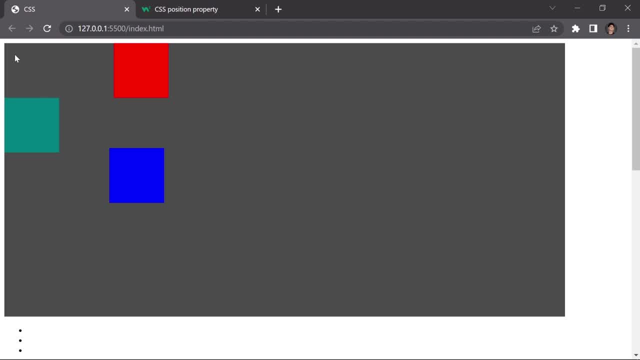 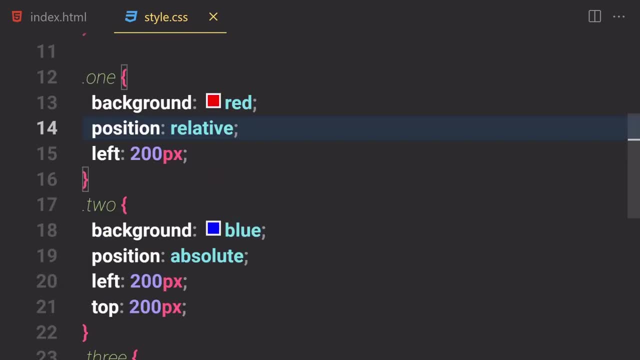 element to anywhere we want, but it will not leave its place. so we will have that same space inside in our Dom, but we can move around this element to anywhere we want. on the other hand, we have position absolute. a position absolute will also allow us to move our element anywhere we want, but 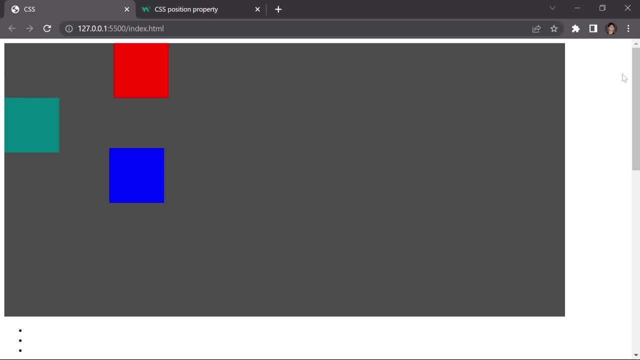 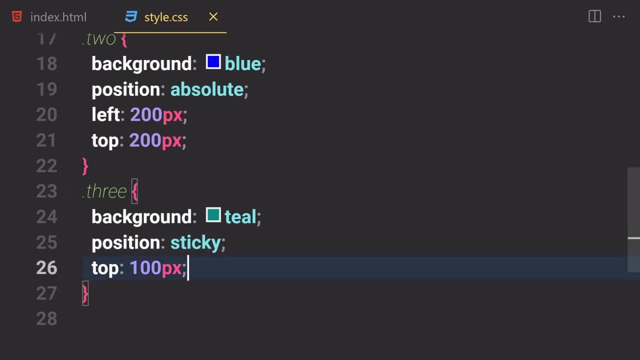 and then, finally, we learn about a fix which will be just like fixed to anywhere we want, and if you scroll, so that element will also scroll with us, okay, and then, finally, we just learn about a sticky property, and sticky will be just like sticky at some place and if you just scroll, so it will just 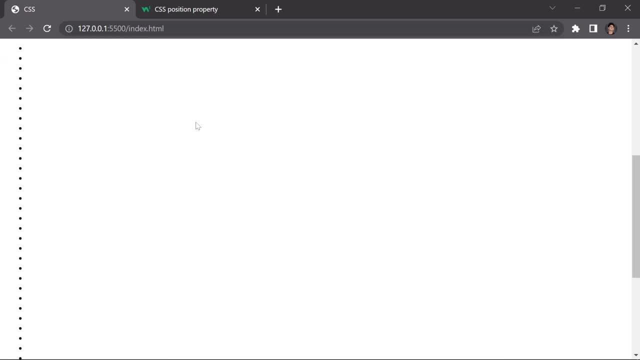 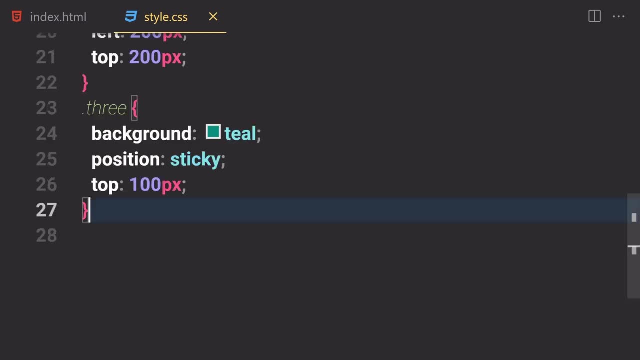 also scroll with us, and when it hit its certain points, it will just stop scrolling. okay, so these were just a few properties which I kind of want to show you in this video or in this section. so now we are totally done with this position property. now the next thing. 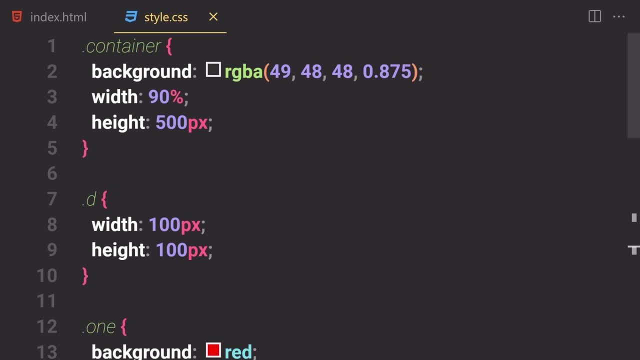 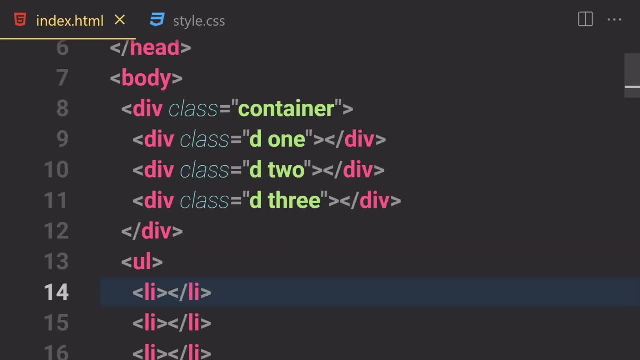 we are going to be learning is called flex box or second position property. so we are going to be deleting everything we have inside our CSS file and now I'm going to save that and I'm going to also delete everything which we have inside or body. I'm going to remove all of that and I'm 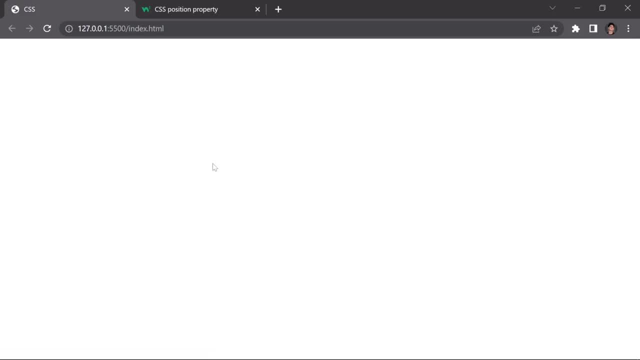 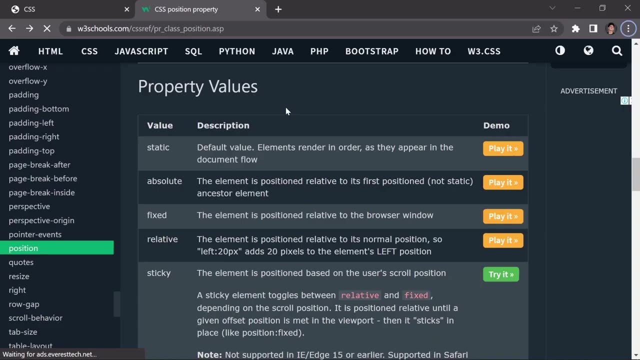 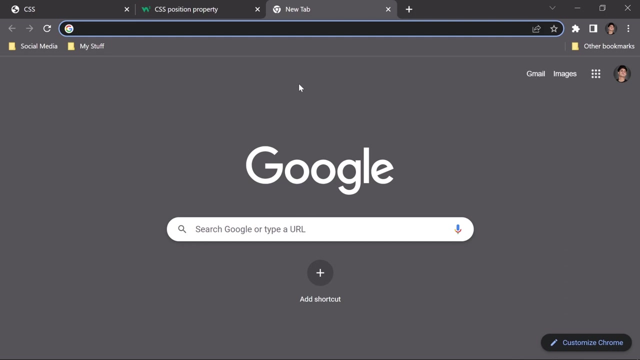 going to cut then and now, if you save that, so we just have our blank body right here. all right, so now let's just start working on a flex box. so for this section, we are going to be heading over through somewhere else called MDN or Mozilla developer Network. so what we have to do, we just have to write MDN, and now here. 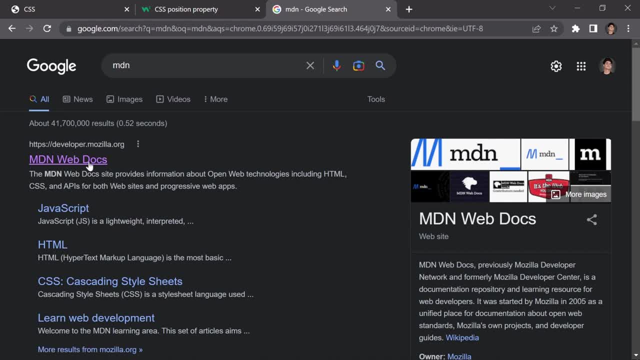 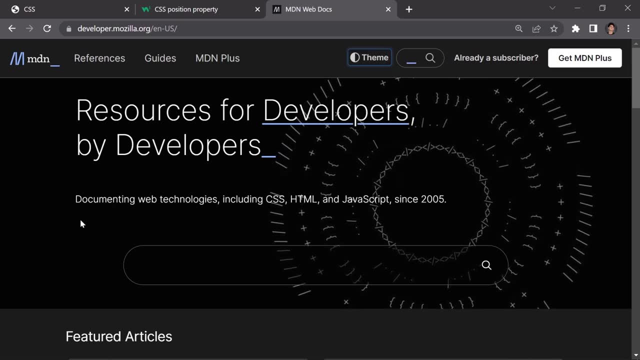 you can see the link. like, we have developermozillaorg and I'm going to click on the first link and you can learn more about that if you want to. you can change the theme if you want to, but in my case I'm not going to do that. documenting web technologies, including CSS, HTML and JavaScript. 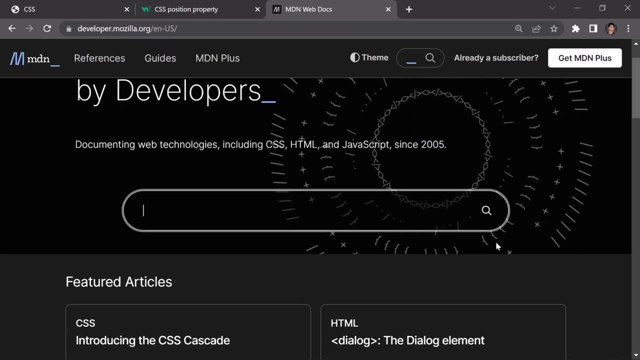 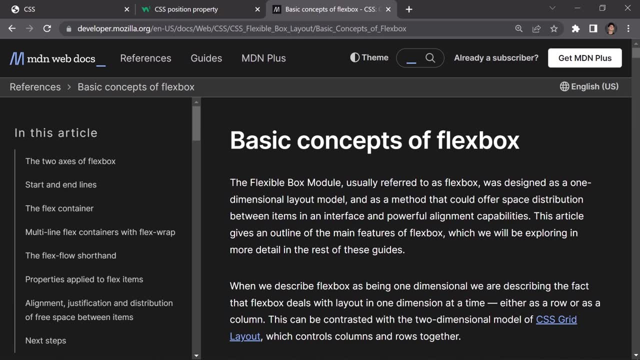 since 2005.. oh, my goodness, okay. so now let's just ask from him: like, what is a flexbox brother? so he works? module usually referred to as a flexbox was designed as a one-dimensional layout model, so flexbox only work on one dimensional load. uh, for either from a left to the right, from the right to 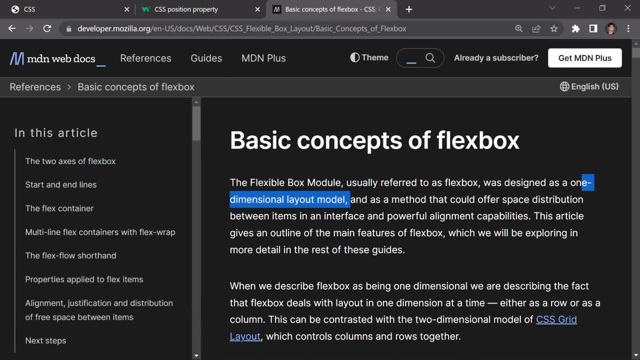 the left, or from the top to the bottom, or from the bottom to the top, which I'm going to show you just in a second. so as a method that could also offer a space distribution between items in the interface and powerful alignment capabilities, and in this article you don't have to work with him for now. so 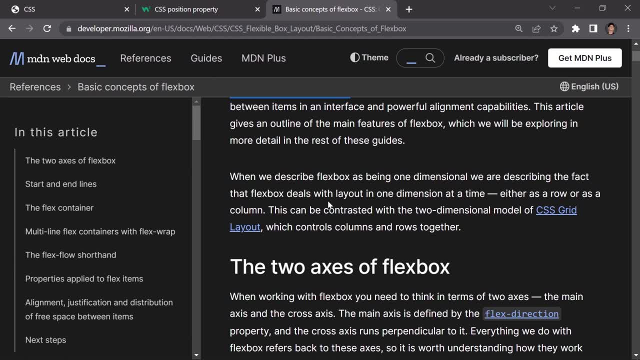 again one-dimensionally. we are describing the fact that flexbox deal with the layout. okay. so if you want to work with the layout, so if you want to push some item from one place to another by either using a row or a column, so for that we can use flexbox, and a flexbox is something which will 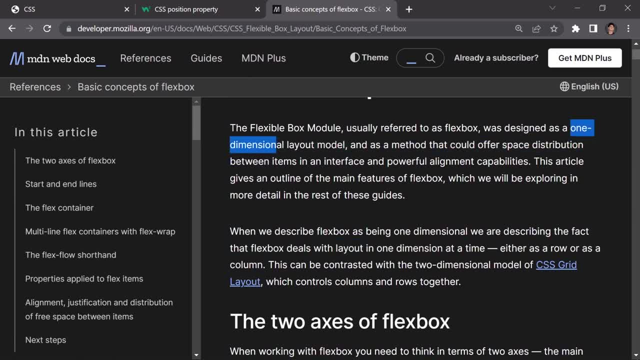 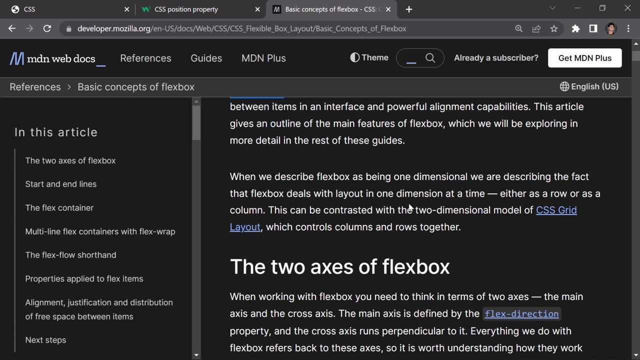 help us with layout, and it will just help us with one dimensional layout. if you want to work with more than one dimensional layout, so for that we have CSS grid, which we are going to be also learning in this video. okay, so, and da, da, da, you can learn more about. 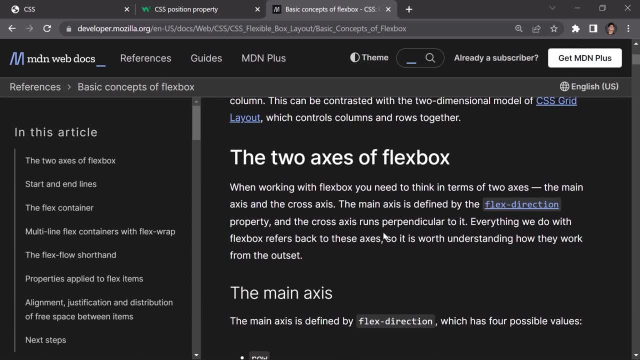 there. so, before getting into the actual coding of a flexbox, you just have to remember two things. so the two axes of a flexbox. when we are working on a flexbox, you need to think about in term of axes: the main axes and the cross axes. so the main axis is defined by the flex direction which we 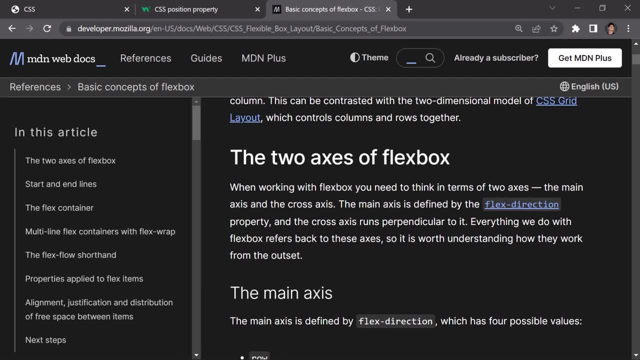 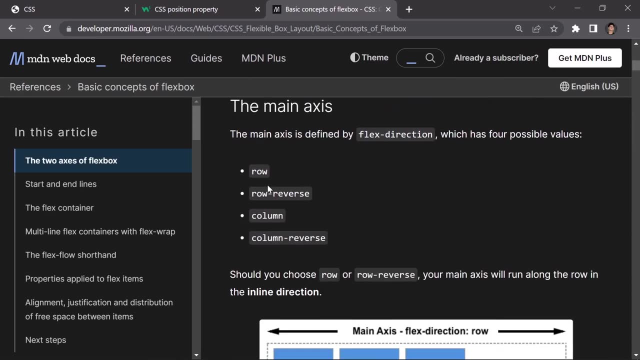 will see just in a second property, and the cross axis runs perpendicular to the flex. um, what do we call the main axis? okay, so everything we do with a flexbox refer back to these axes. so it's worth learning about flexboxes. so, the main axis we have these properties which we are going to be. 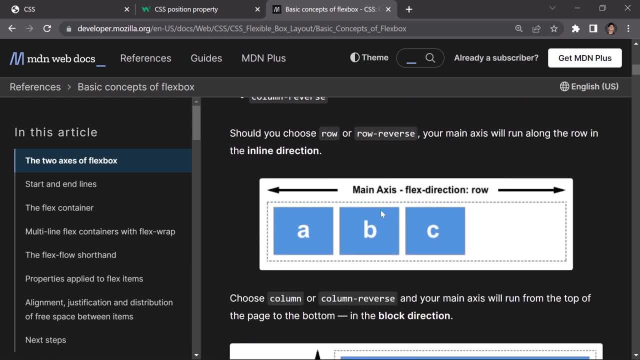 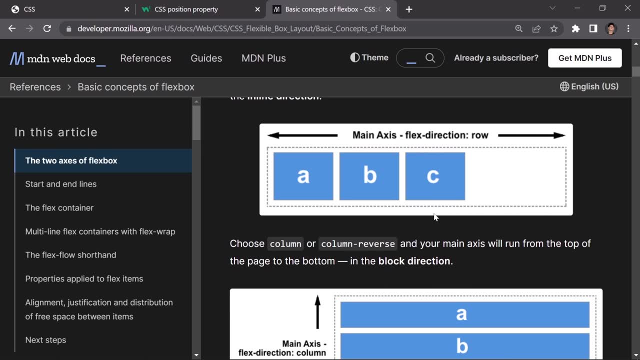 exploring. so if our main axis is set to the row, or cross axis will be set to the column, because cross axis will be perpendicular to the main axis. so for now you just have to remember that. and now let's get into the coding. so, by the way, let me just say that one more time so that you guys don't. 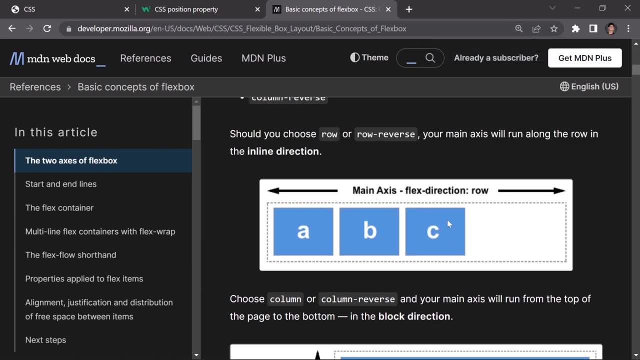 get confused: if our main axis is row or cross axis will be column, like our cross axis will be perpendicular to our main axis. okay, so i just said that one more time, and now let's get into our coding. so now let's just start working on a flexbox. so the first thing we would do is that we have to 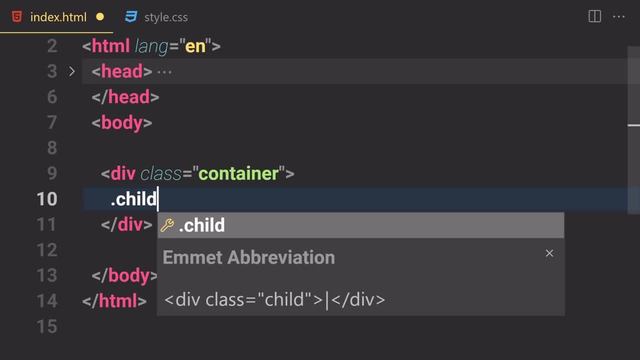 first of all, create a container. inside this container, we are going to be writing a lot of children's like child, and we are going to be writing like: uh, i don't know i'm going to use emit, uh, we have a child, and here let me just write a dollar sign and boom, and how many we want. we. 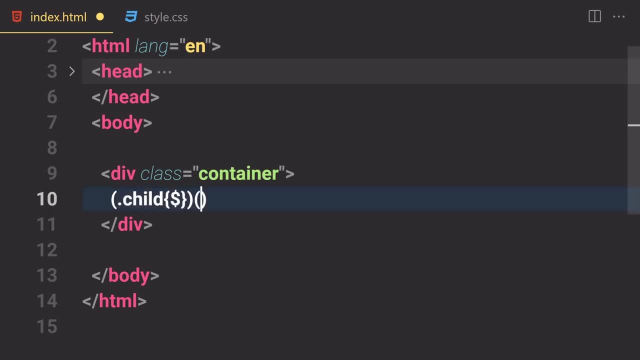 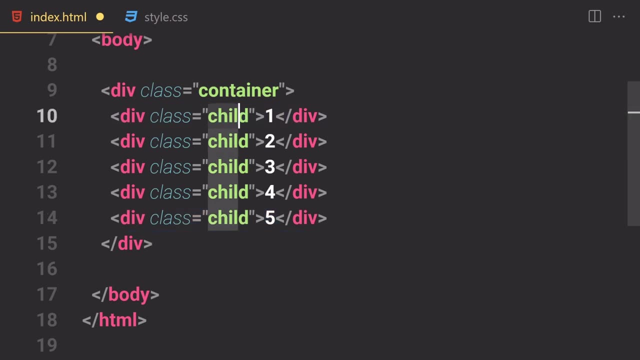 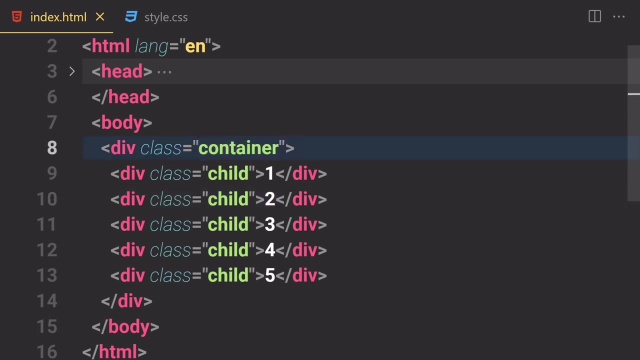 want them to be like: uh, i don't know, maybe five for now. so we got like one, two, three, four, five, and each of these day will have a class of child, okay, so before working on a flexbox, you need to remember a concept called containers. so if you want to work with a flexbox, like if you want to, 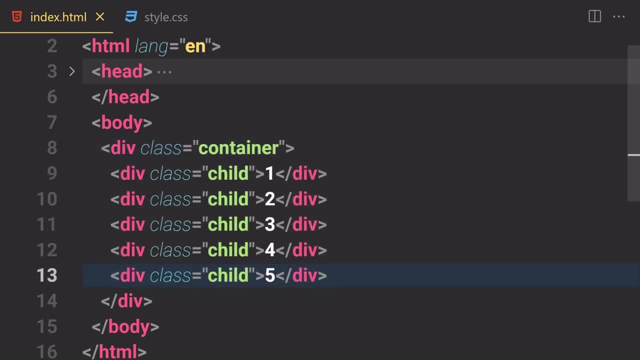 move around these uh children's. so first of all you have to target the container. you cannot work with a flexbox inside a children's. you would work on a flexbox inside a container container. so if you want to work with a flexbox, first of all you have to select the container. 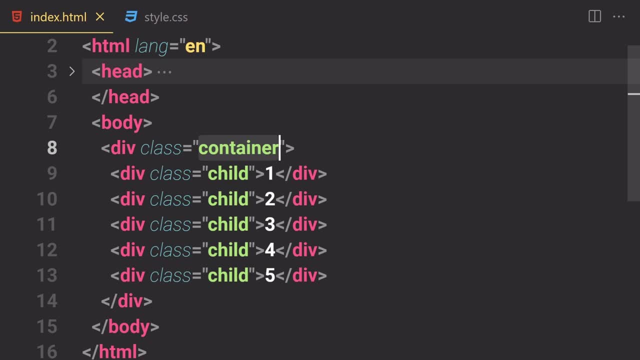 it doesn't matter. like whichever kind of container you have, you can also call it like a parent. first of all, you have to select the parent, and you can work with a flexbox by using a parent or container where you want to call it. so now let me just ask you a few questions. first of all, uh, i'm going to 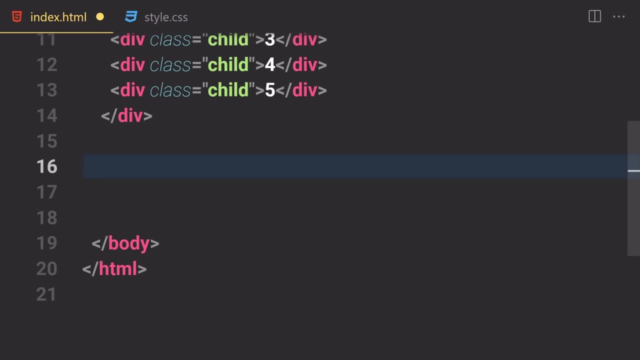 just write like a little bit coding so that i can tell you like what is a container or parent and stuff. so let me just write a section. then inside this section we are going to be writing our article. inside this article we are going to be writing a ul and then we are going to be writing: 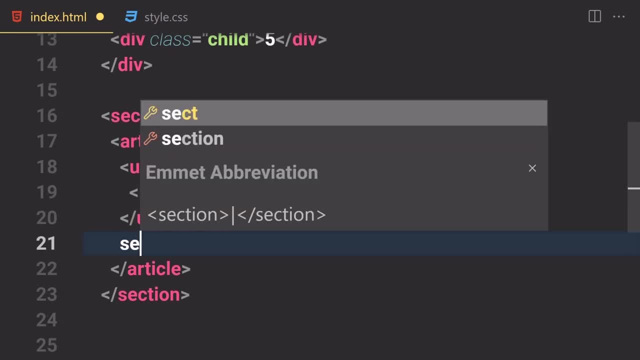 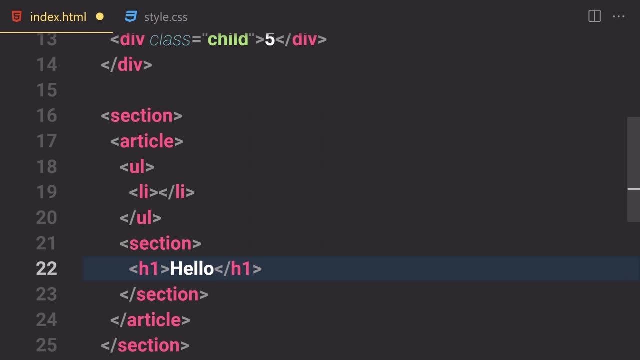 li, and then, outside from this ul, we are going to be also writing another section, and now, inside this section, we are going to be writing h1 of hello. okay, so now let me just ask you a question: what is the parent of this h1? i want you to answer? i want you to answer that. well, the parent of this? 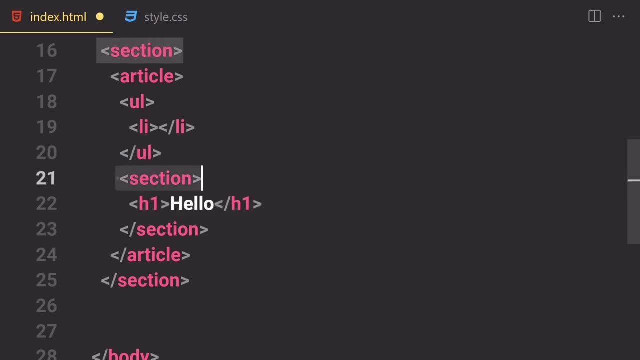 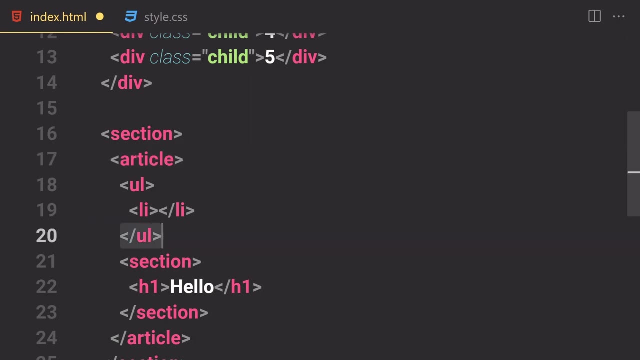 h1 will be this section, not this one, but this one. so what is the parent of this section? the parent of this section is this article, not a ul, but an article, because this is the parent. okay, these two are the nested children of this article right here. so what is the parent of this article? the parent of this article is: 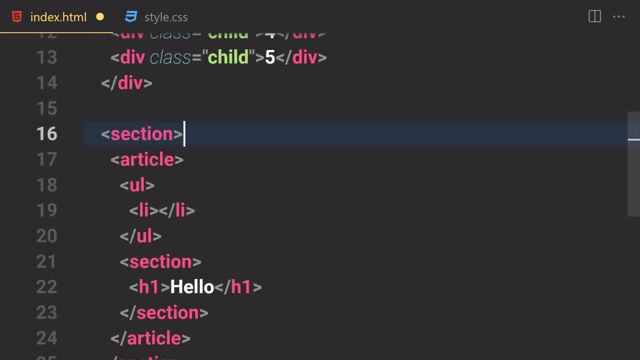 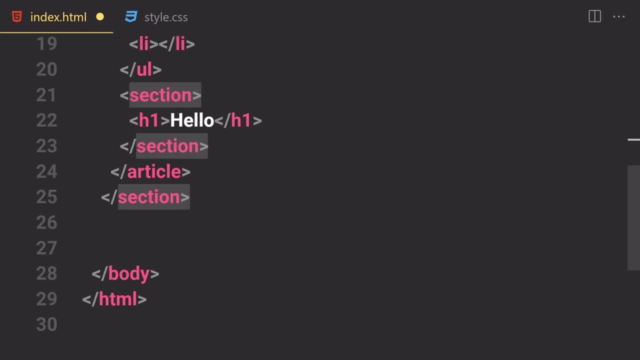 this section. so now, if you want to work with a flexbox, so first of all we have to provide, first of all we have to set a display of flex on this one, and all of these item will just go on and on. so i'm going to show you all of that just in a second. so i just kind of want to give you. 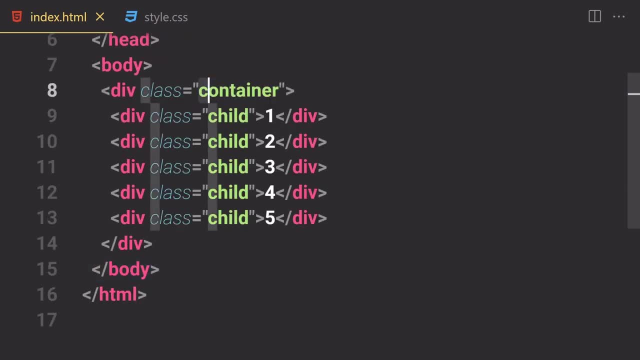 this test. i'm going to remove that. and now, here you can see, we have this container and you know what. i'm going to change this one to section, to be precise, uh, so that you guys can see everything. so i'm going to just write section and then we have a div with a class of child and 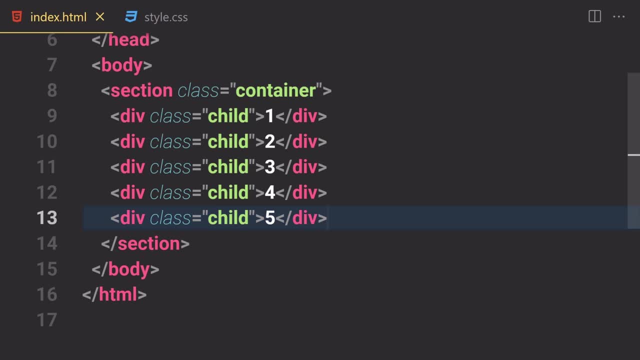 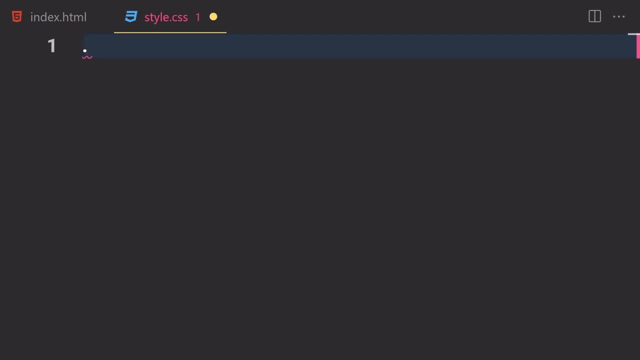 we have from one through five right here. okay, so if you want to work with a flexbox, first of all we have to target a container. so let me just write a little bit of formatting and then we are going to start working on our flexbox. so i'm going to just write a container, or before getting into 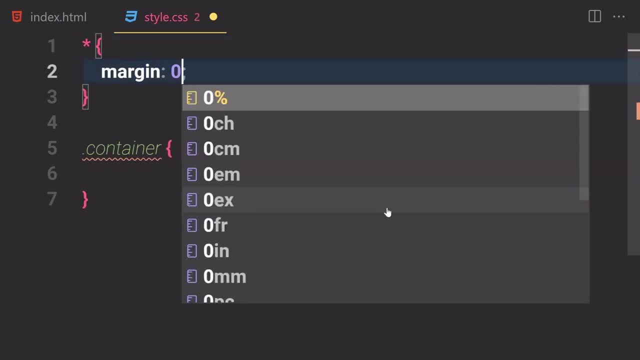 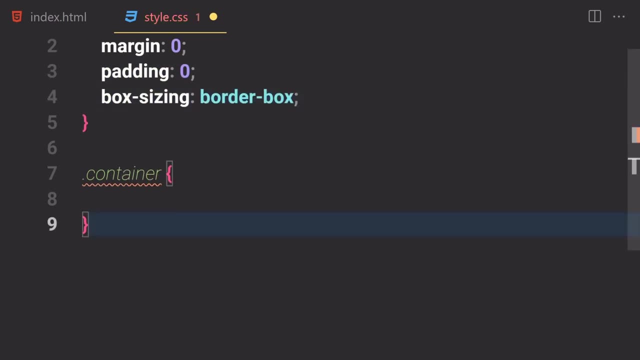 the container. we just have to remove or reset first of all. so i'm going to just write margin and padding of zero and then i'm going to just write like a box, sizing of border box right here, and you know what. i'm going to remove this border box and stuff. for now let me get my body, and inside this body we. 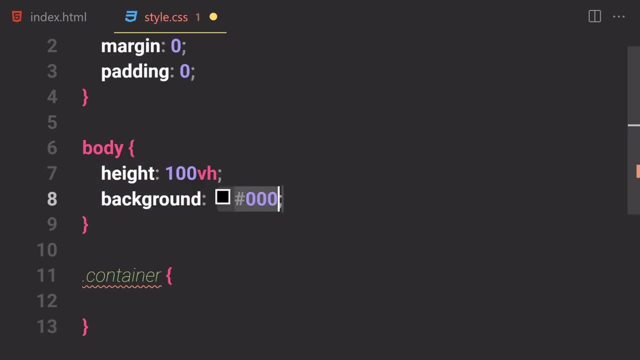 are going to be writing a height of 100 vh and i'm going to provide a background of this kind of like a blue violet color, like blue violet. i'm going to select that now inside this container. what do we have to do? we have to first of all write a border of two pixel, solid and totally. 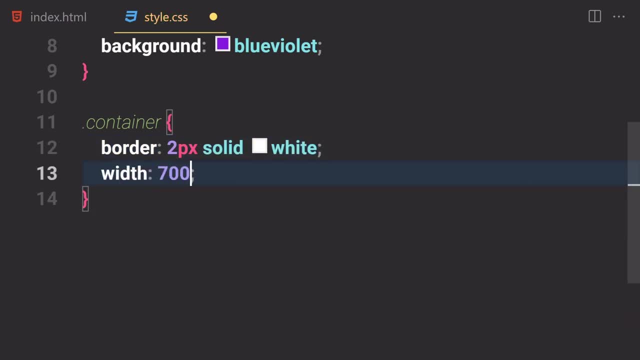 white. and then let me just provide a little bit of width, like, uh, 800 pixel would be fine. i'm going to provide 800 pixel of width and i'm going to also provide a height of like 400 pixel would be fine. okay, and then i'm going to also provide a margin of 20 pixel, and 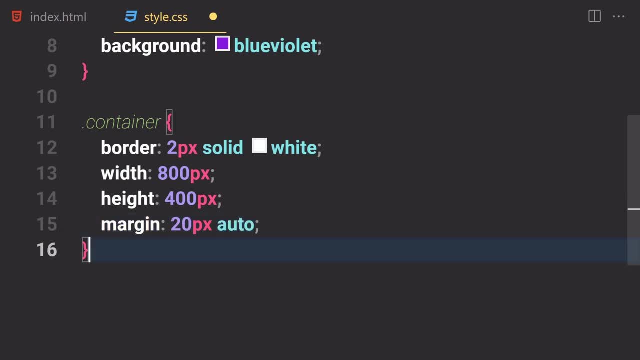 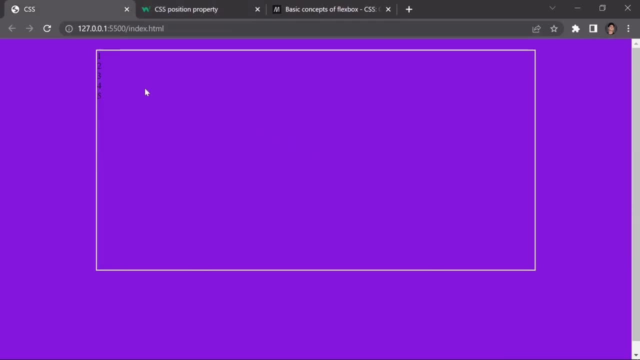 auto, and auto will be just uh, automatic stuff. okay, now let me just save that, and this is how my file will look like right here. so now the next thing which we have to do is that we also have to uh format these divs which is inside this container. so we are going to be formatting there by using our 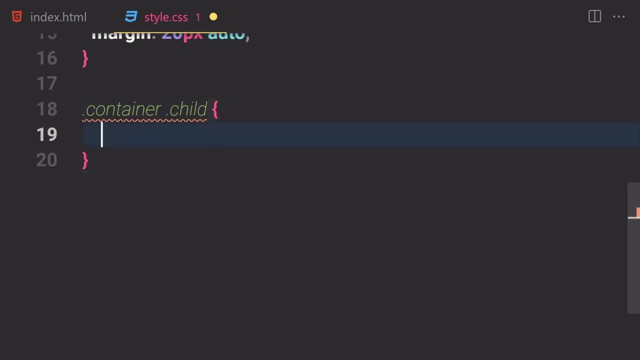 container and now let's just get our children. so i'm going to write a child right here and what we have to do. we have to give them a little bit of width of 50 pixel and i'm going to also provide a 50 pixel of height to it. background color will be like you can give them, whichever kind of. 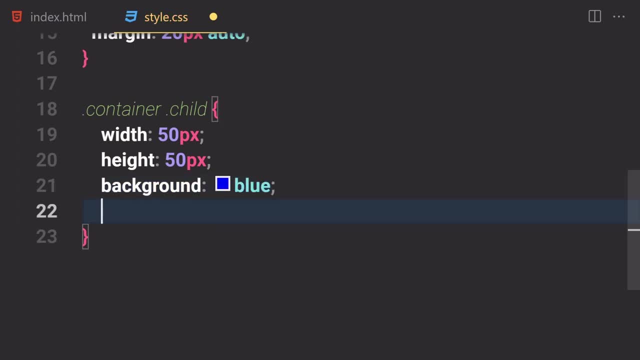 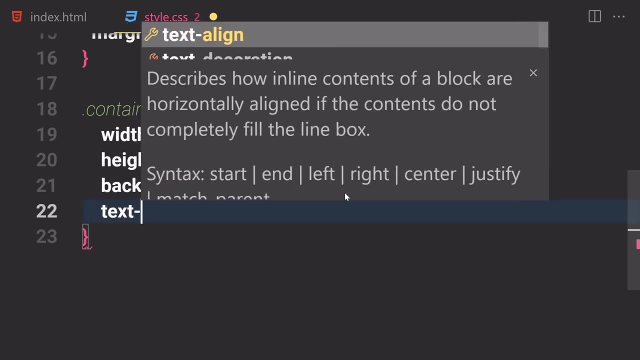 background color you like. in my case, i'm going to set that to blue and i'm going to also provide a font family of not font family font. uh, nah, i'm going to just write text, a line of center, and i guess that would be it. so if you save that, this is how things currently look like, but i just felt. 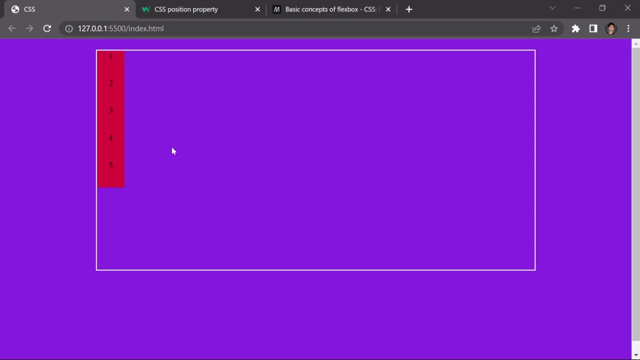 it's a little bit, uh, low contrast. so if you save that and now i guess everything looks like a bit better. so i'm going to just write a bit of margin, like 10 pixel would be fine, and if you save that and now we are cool. but i guess instead of 10 pixel i'm going to provide 5 pixel margin. so now, 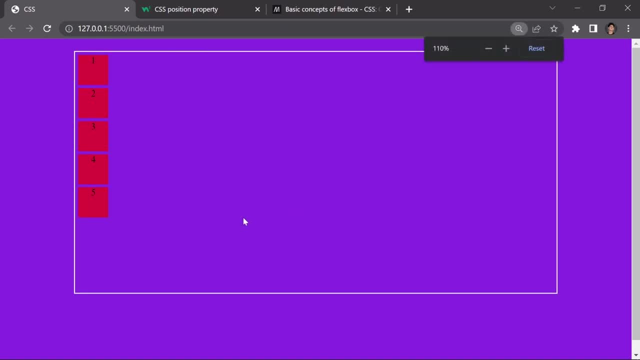 we're good to go. and so now, if i ask you a question like: what will be the container of these elements? so we have now these children, so what do you think will be the container? will it be this body or will inside this container? so now, this is obviously the container, and now we have these children's. 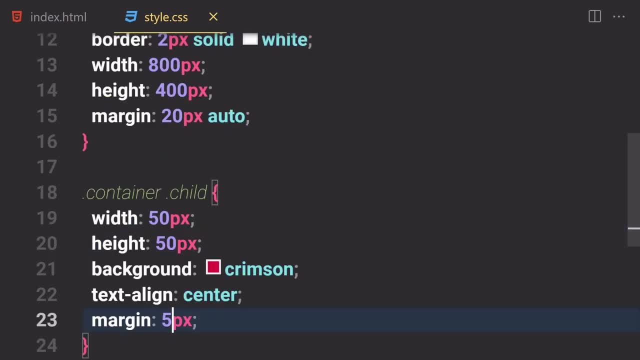 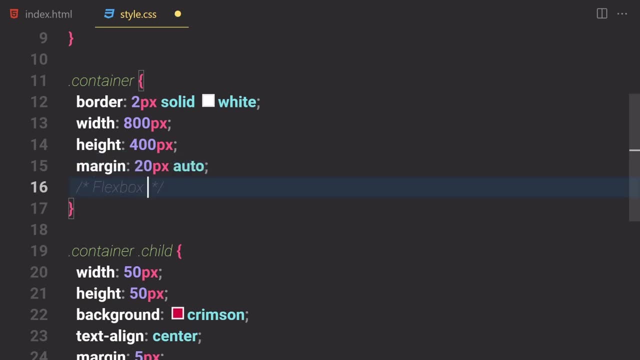 inside this container. okay, so now let's just start working on a flexbox. so i'm going to zoom out a bit so you guys can see everything a bit better, and let me just write a flexbox stuff here. okay, so we are going to be starting our flexbox stuff from here. remember, if you want to work with a 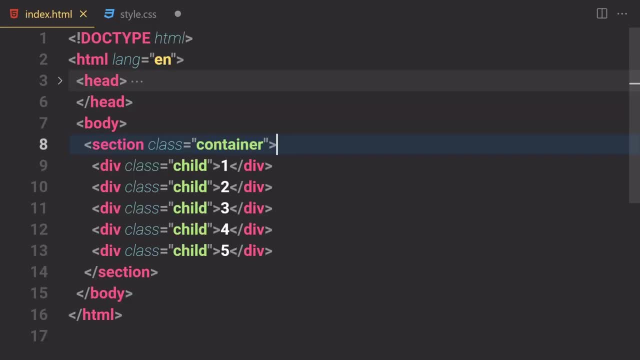 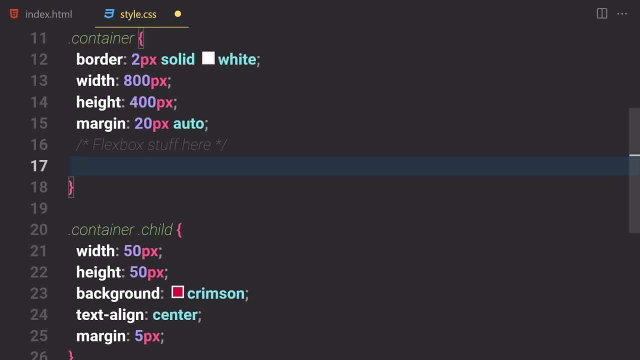 flexbox, so you just need a few things. the first thing you have to remember that you are going to be working on a container. don't forget that. and now, the second thing you have to remember is that. the second thing i want you to remember is that, first of all, you are going to be writing a display. 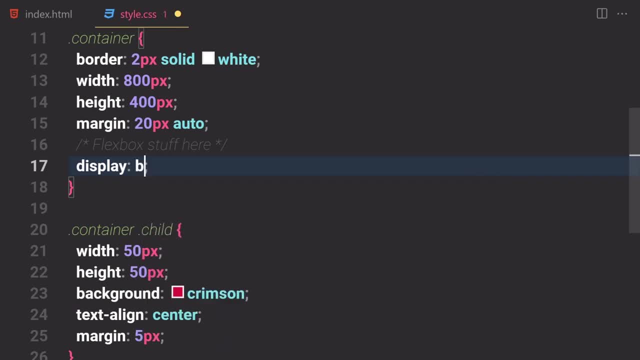 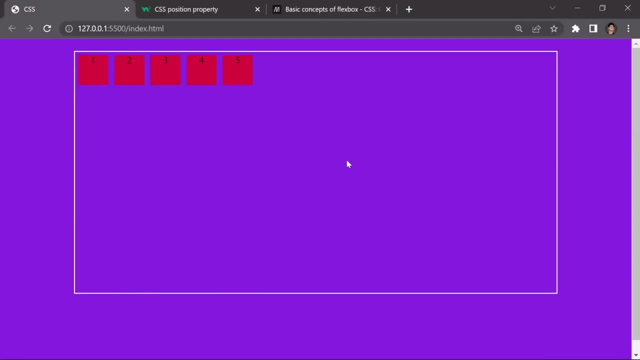 of flex properties. so we already learned about display of block, we already learned about an inline inline block and we also learned about display of none just a second ago. now, in this case, what do we have to do? we just have to write a flex. and now, if we just write a flex and if we save a file and 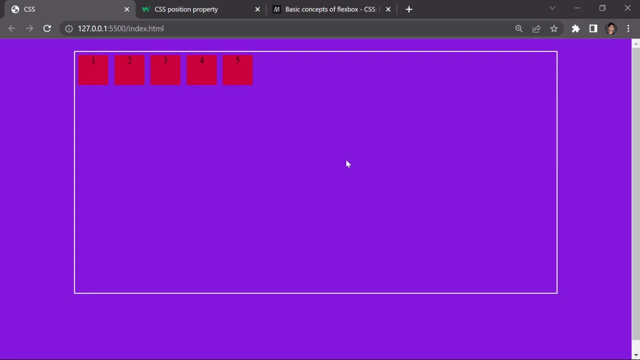 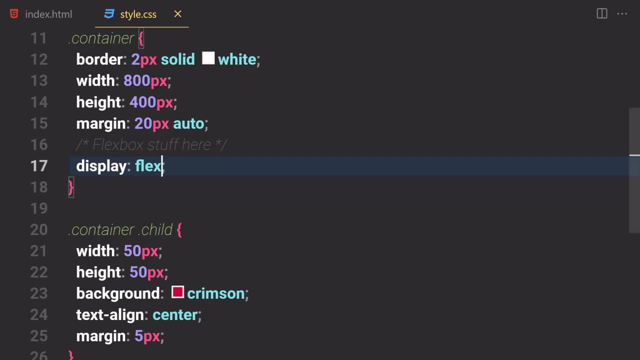 what happened? wow, this magic happens. so by default, if we just write a display flex, so flexbox will provide a display of none. and if we just write a display of none and if we just write a display of flex, we are then going to be using a little bit of styling to our children. so which kind of 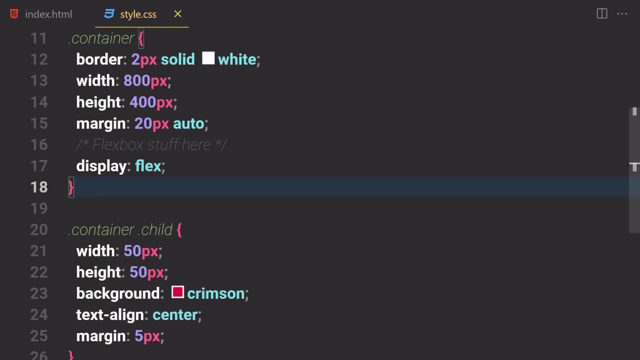 styling. we have like a flex um direction and it will be now set to row. so now, first of all, let's just learn about a display flex. so if you just write a display flex, so first of all it will give us a little bit of styling right here and i'm going to be telling you like which kind of 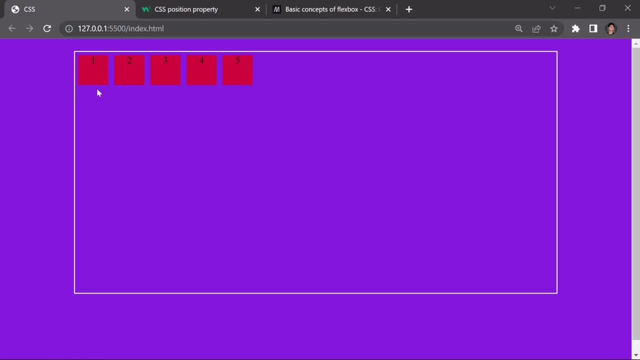 styling by default. display flex provides us, but you don't have to worry about them for now. so now we are now totally working on a flexbox right here. okay, and, as i said, that flex box is one that organisations t talks today. okay, that's three leaves, and there's also the plastics they need, and not just the. 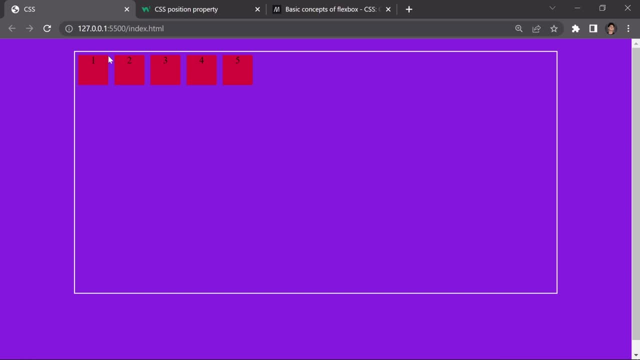 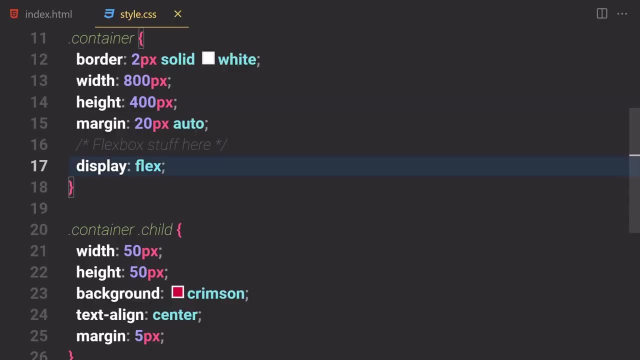 one dimensional layout, so it will just either work on a row or a colon, okay, so you just also have to remember that as well. so now we are totally done. so now the next property which i want to show you is something called a flex direction. so if i just write like a flex direction, 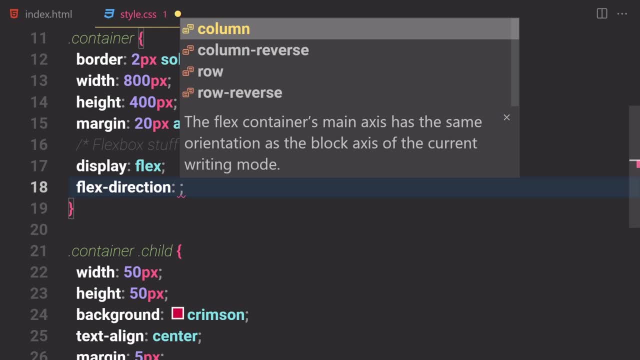 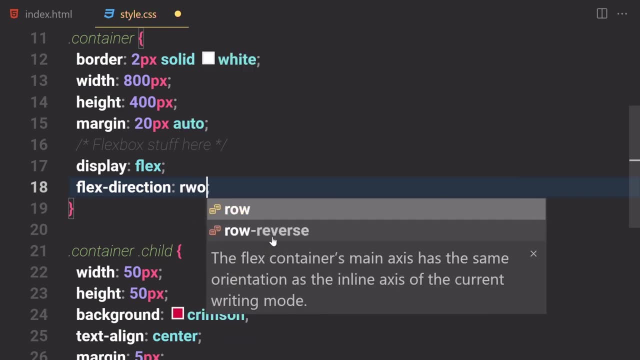 so, as the name suggests, their flex direction will allows us to change the direction of our flexbox. so if you just write a display of flex, by default the flex direction will be set to row. if you just write like a row in here and now, if you save that and here you can see, nothing will happen, right. 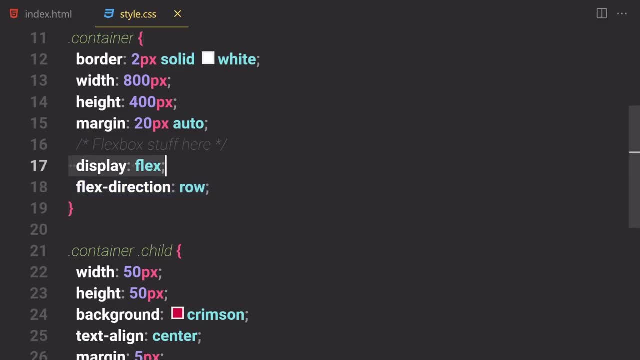 here. why is that? because if you just write display of flanks, so by default this uh display flex will provide us with this flex direction of row. so we can also change that to like colon if you want to. so if you just write colon and if you save that and here you can see, it will now change your layout. 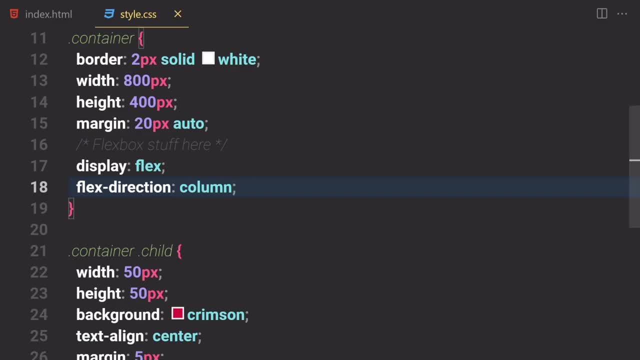 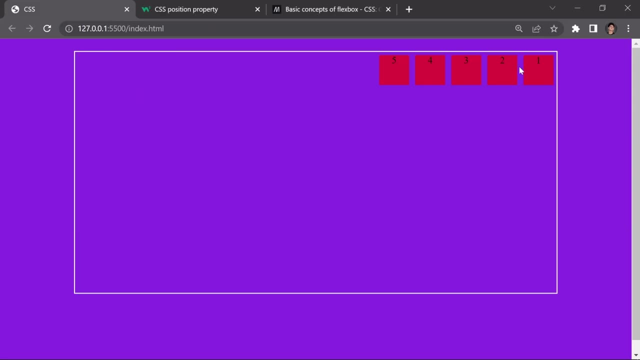 to the column right here, okay. so now i'm going to remove this column. so we have like a row- we already saw row, we already saw colon, but we can also write a row and then reverse, okay. so i want you to notice like we have one, two, three, four, five right here, and if you save that and boom, it will now push it right here and 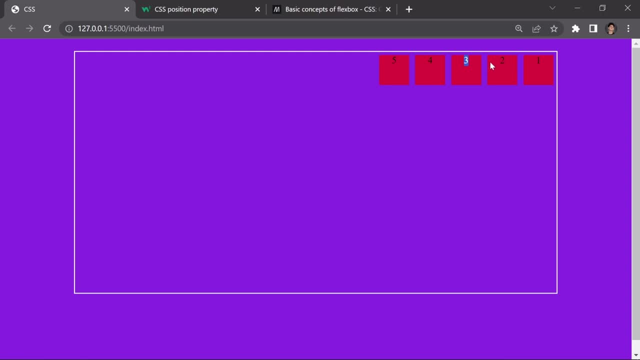 first of all, you will get five, then you'll get four, then you'll get three, then you will get two, then you will get one. so what's happening? so, if you just remove this reverse from here and if we sell that, so here you can see, this is how everything will look like right now. okay, so if 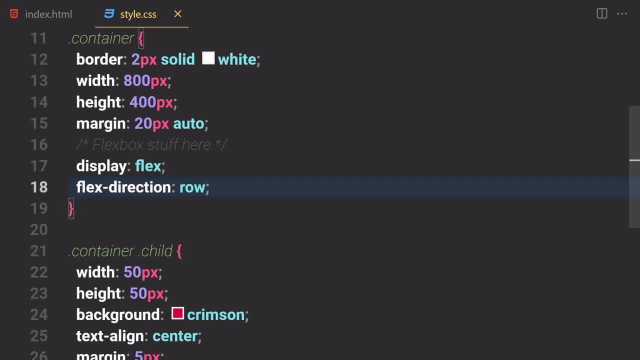 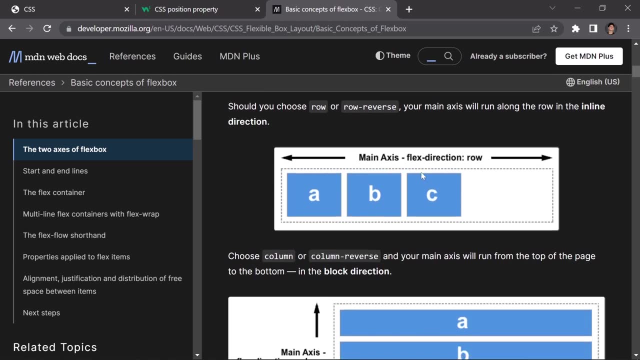 you want to reverse that and also the direction of it. so for that we can just write like a row and reverse. okay, as i said that if we're main axis, uh, okay, so if our main axis is set to row or cross axis will be perpendicular to that. 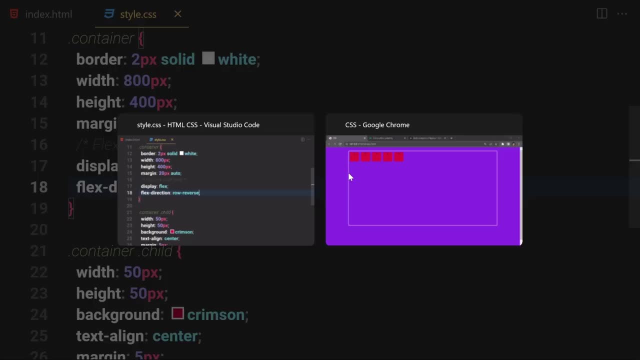 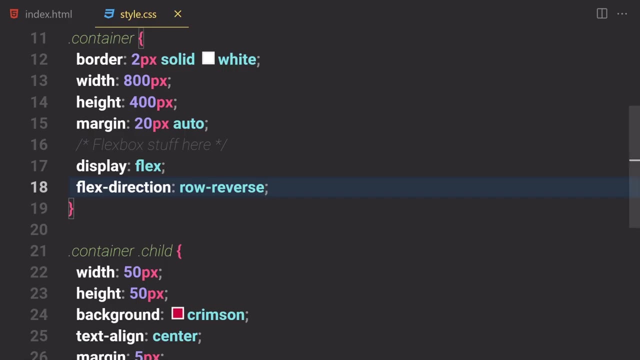 so this is how we can get that uh kind of effect. so if you sell that and boom, or level is changed to the row reverse right here. okay, so this is how we can change that. and we can also change this to a colon reverse, if you just write colon and then we have reverse. and now if you sell that, 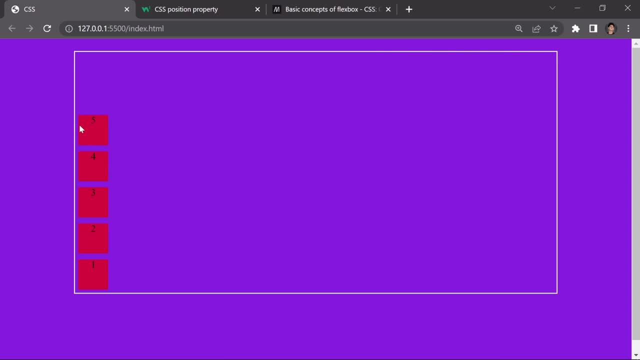 and here you can see, everything is pushed up to the bottom right here and we have five, four, three, two, one instead of like one, two, three, four, five. so if you want to just remove that, reverse, and if you sell that, what do we get? we get one, two, three, four and five, and i guess i should have to make 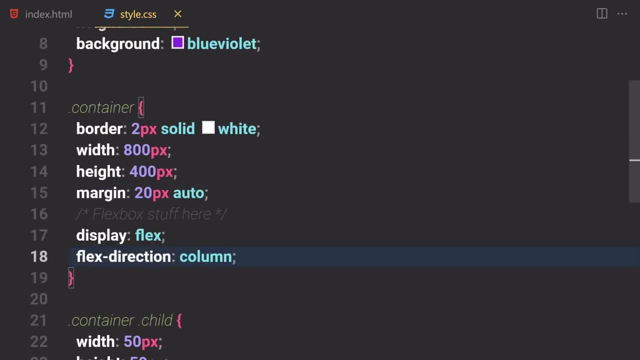 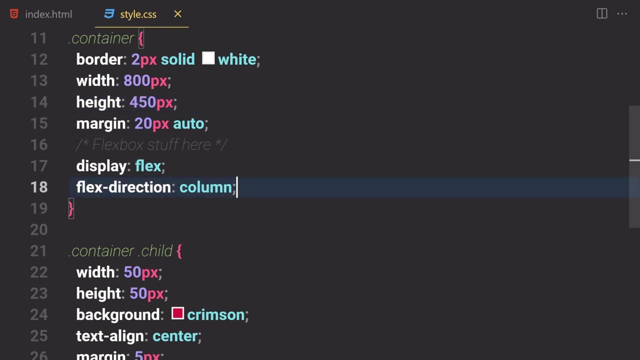 this one a little bit bigger so that you guys can see everything a bit clear. so i'm going to put a little bit of more uh higher towards the 500 pixel would do, or you know what? uh 450 would be fine. i guess that's going to be fine anyways. so this is a flex direction. first of all, we just 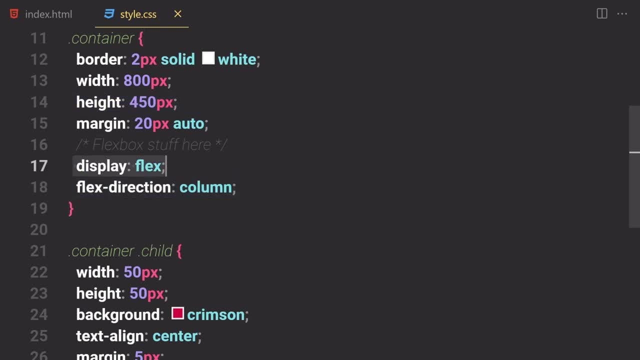 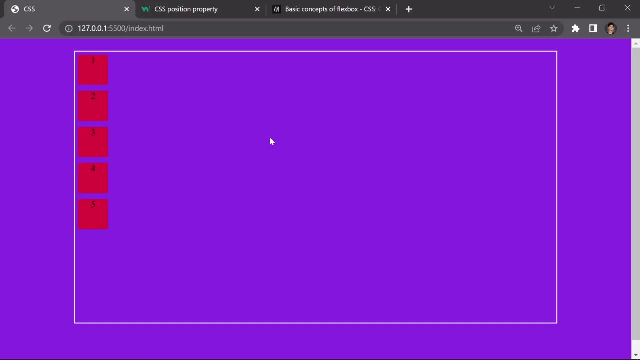 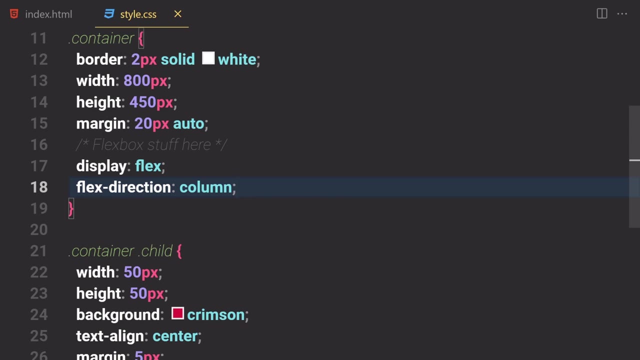 display of flex. and then we learn about a flex direction and it allows us to change the direction of our layout. okay, so it will just work, um, on a flex container and it will change our children. so you just have to remember these things in mind. and now, what else do we have to do? uh, we are going to 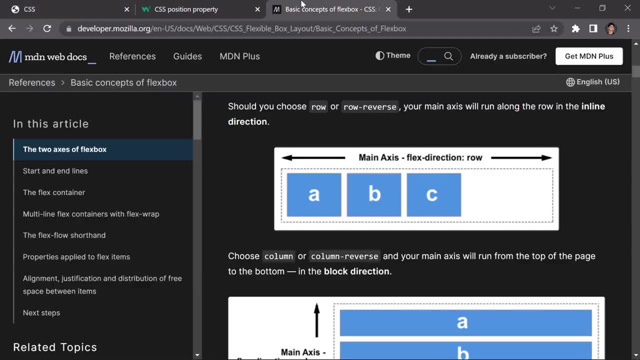 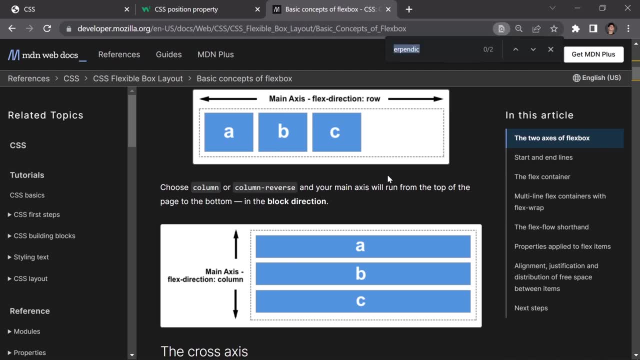 be learning about a justify content property. so for that we have to ask our good old friend: like: what is a justify content property? so i'm going to just hit control space, not a control space, but just a control and f. and now here i'm going to just 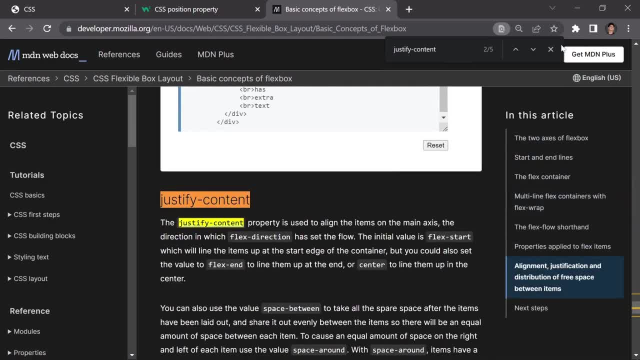 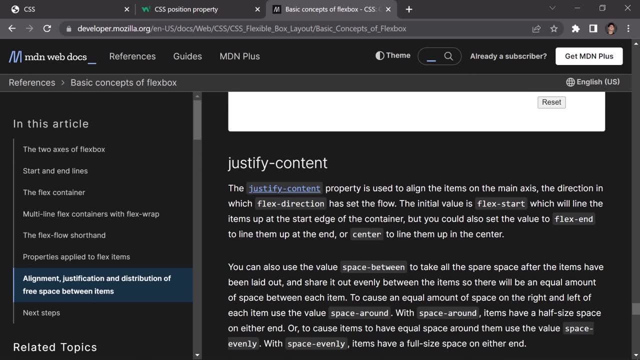 ask for like a justified content. if i just write justify content, so it will gives us this definition. let me just zoom in a bit. and now, here you can see, the justify content property is used to align the items on the main axis right here. so this justify content property will be responsible. 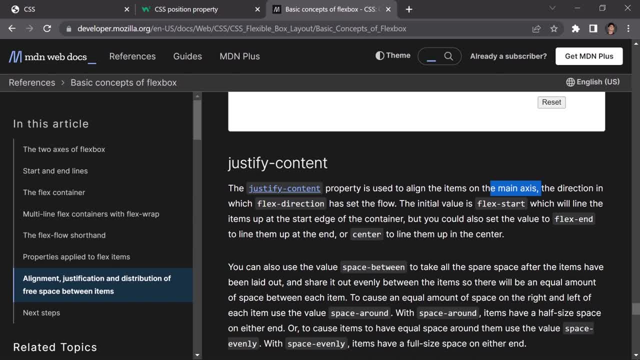 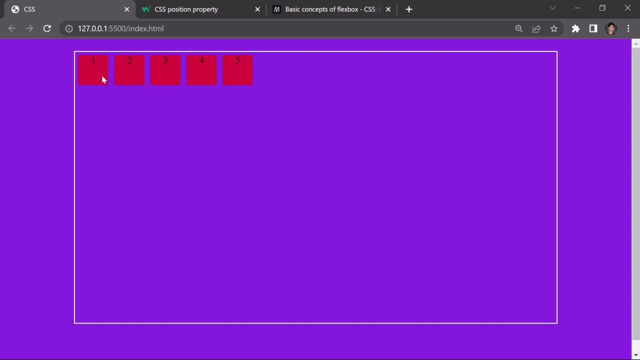 to align our item on the main axis. so how can we go about doing that? so now, instead of just column, i'm going to just comment this line out, and if you save that, everything is now back to the row right here, and if you want to push this item to the end, so we're going to just click on this. 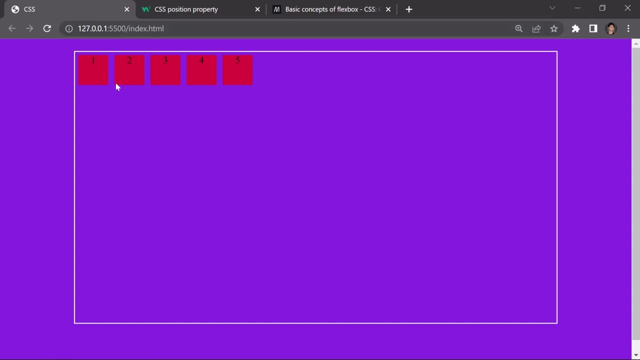 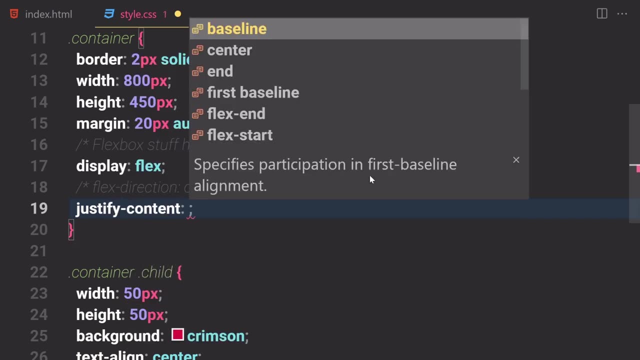 can also do that, we can also make it center, or we can also just stick it right here. so now let's just learn about something called justify content. okay, so justify content. by default, the value will be: um, what do we call it? flex start, so the default value of justify content. if you just write a, 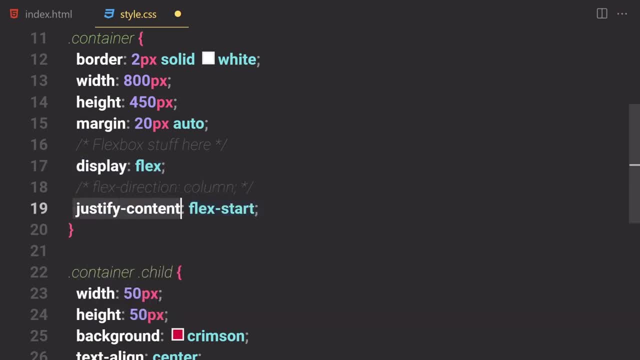 display flex. so the default value of justify content will be set to flex start. if you save that and nothing will happen right here, and we can also change that to flex, and if you want to, so i'm going to just remove that and if you hit ctrl space, it will now give us all of these values. 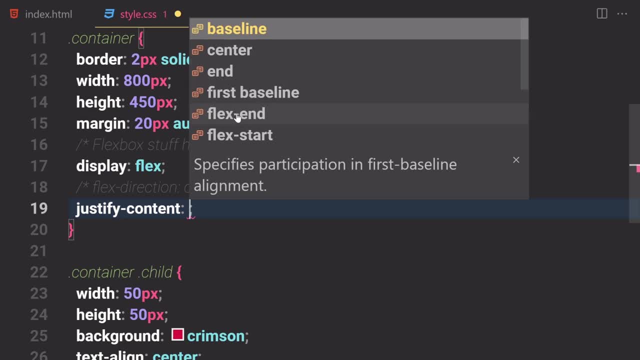 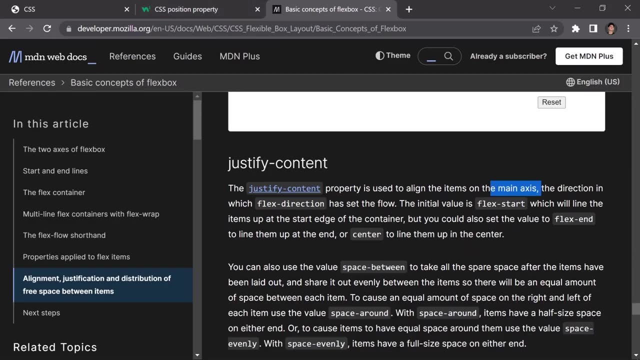 right here. you can use a shorthand like and and start if you want to, but by default it will be set to flex start. we can also change that to flex end, so as we learn that, it will just only work on a main axis and our cross axis will be perpendicular to our main axis. you just have to remember these. 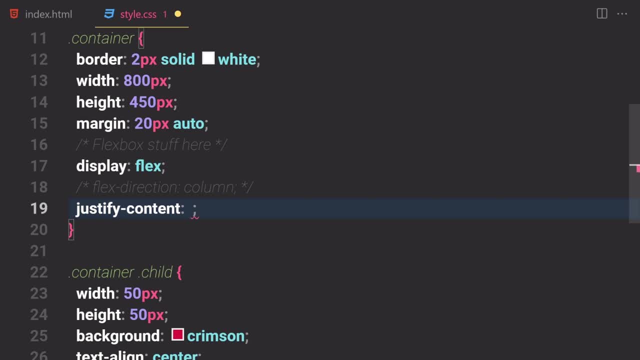 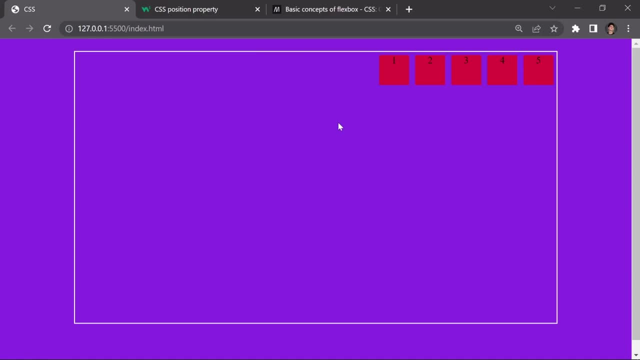 kind of stuff in your mind. so now, if you want to push that to the left, and so i mean like to the right, so for that you can just write like flex and then end. and if you just write a flex, end, and if you save that and boom here you can see that it will now push it to the left. uh, 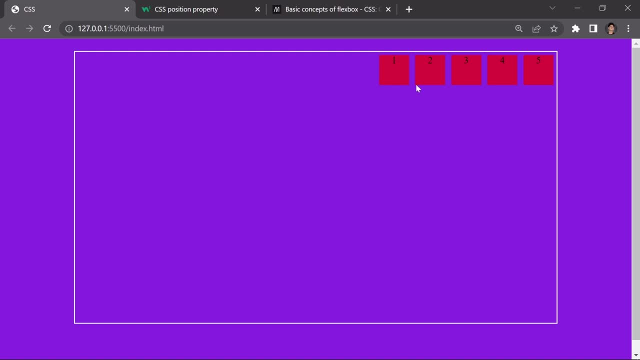 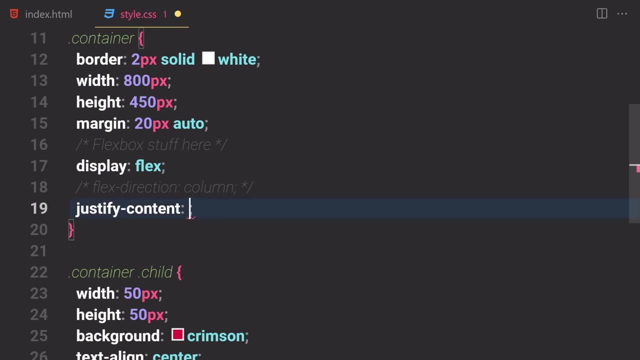 why am i saying left? it will now push it to the right, right here. okay, so that's how we can work with the justify content property, but we have a little bit more stuff in there so we can also make things to the center. so if you just want to write like center and if you save that and here, 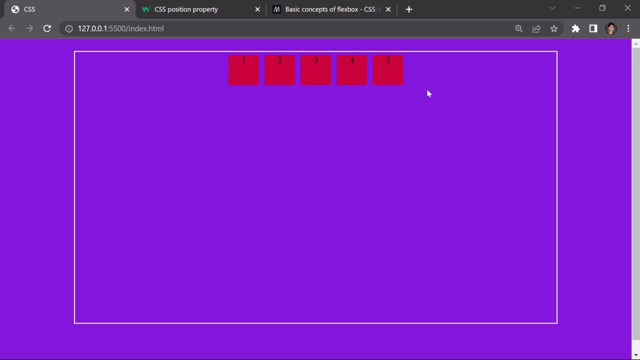 you can see it will now make it perfectly center right here. okay, so now our flex direction is set to row, so this is how everything will look like: like we can center it to the right and stuff. but if you want them to be at the column, so we can also. 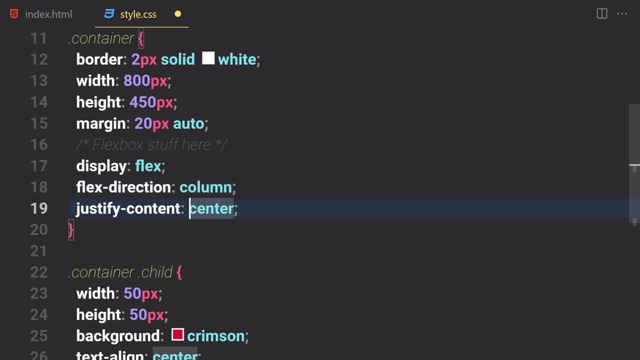 change this flex direction to the column and we can also make it perfectly centered on the column as well. so if you save that and boom, and this is how everything look like and you can also write just like a flex start. and if you save that- and this is by default- we can also change that to flex. 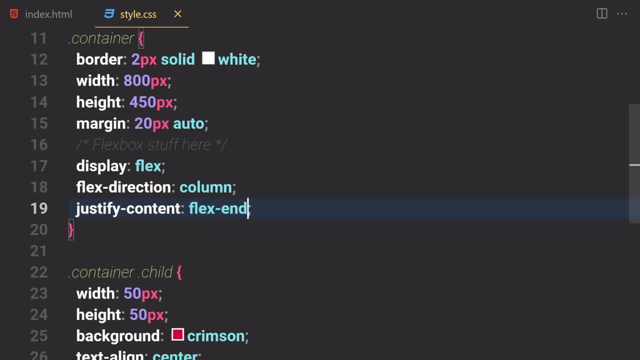 end and if you save that, so this is the flex end and we also saw a flex center. okay, so if you save that, certain log uses that. so let's just check a little bit more about that. so let's just check a little bit more property of that, so we have baseline. you don't have to worry about that. so 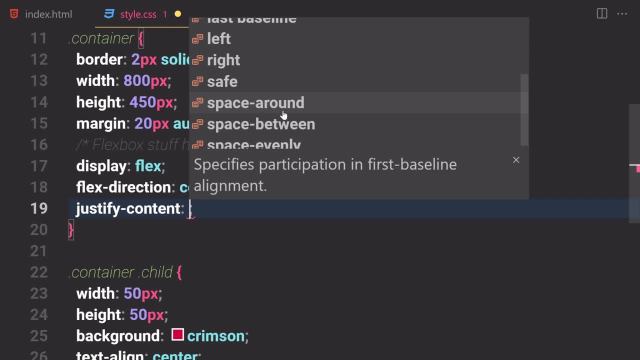 the next property which i'm going to be telling you is something called a space around. so for that you know what i'm going to comment this line out and if you save that, so by default everything looks like this. and now, if i just use like space and around, and as the name suggests, that it will. 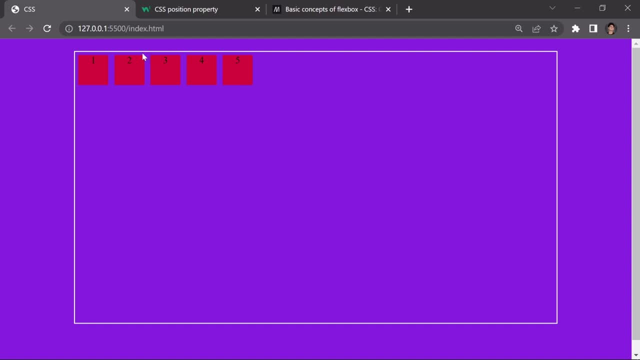 distribute or items like over children, and it will provide a little bit of spacing in there and it will also provide a spacing around these items. so if you just save that and here you can see, it will now distribute your items and it will also provide a spacing. 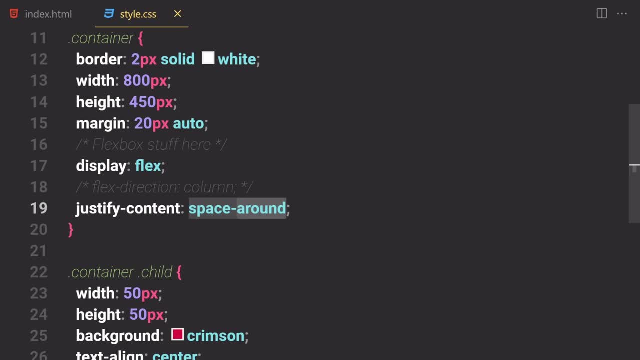 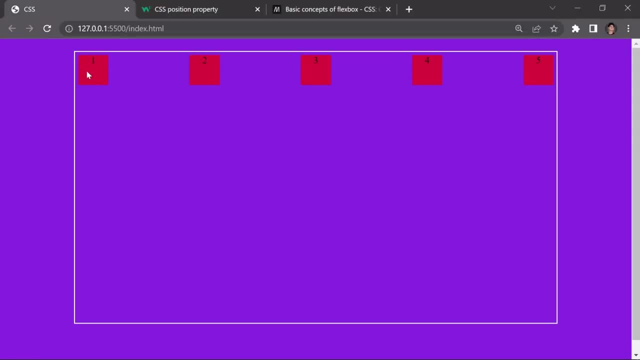 how much they need. now, this is a space around property. we can also write a space between if you want to. so now here, they will not provide a spacing in there. so if you just save our file and here you can see, it will not provide a spacing around that. and if you are wondering like: 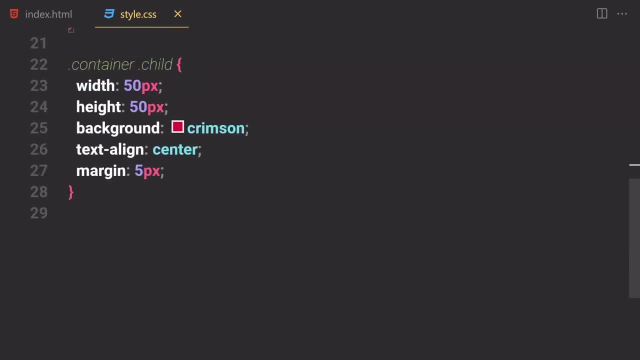 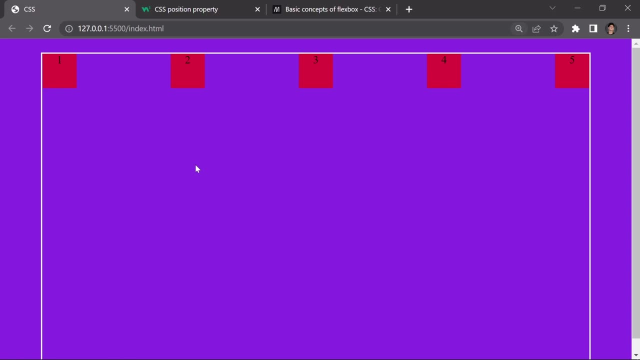 we do have this spacing right here. that's because i've provided a spacing or the margin of five pixel right here. so that's why we are getting this a little bit spacing in there. we just remove that file here, you can see that spacing is gone. so that's kind of a cool stuff, so we can also go. 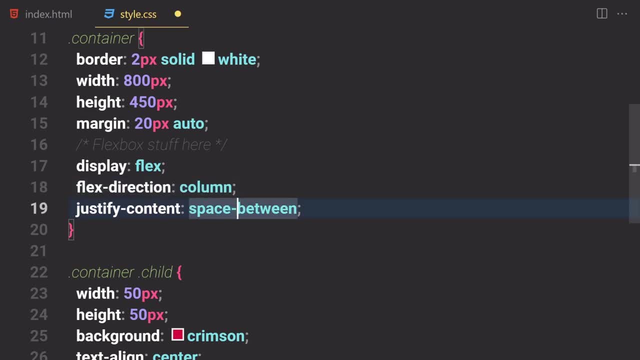 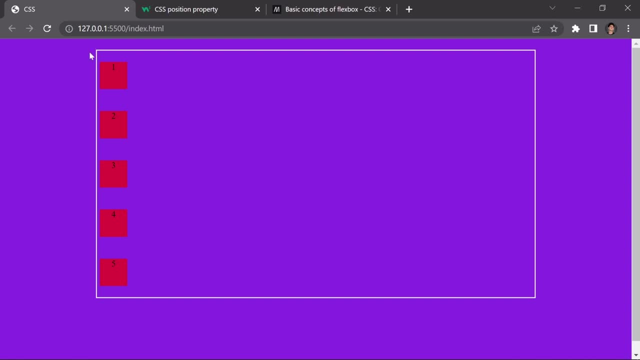 with the flex direction of colon and we can also write a space between. so if you save that and this is how everything will look like, and if you just change that to around, and if you save certain long uses, this spacing around this item right here. okay, so that's it about justify content stuff. 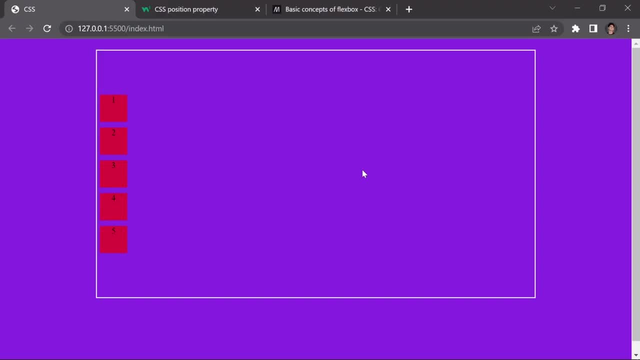 so what do i have to do? i'm going to just write a center right here. so if you save that and it will now make everything to the center, so i'm going to comment this line out. i'm going to also comment this line out. okay, so now the next property i want to talk to you about is something 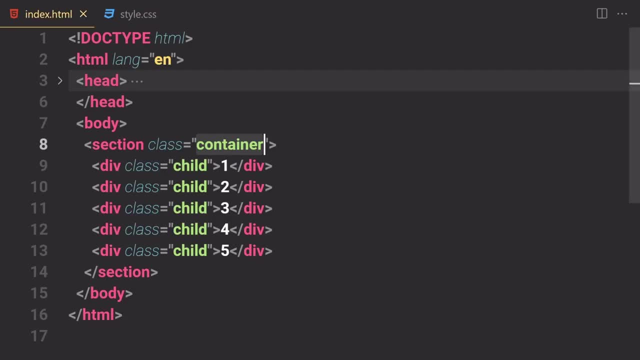 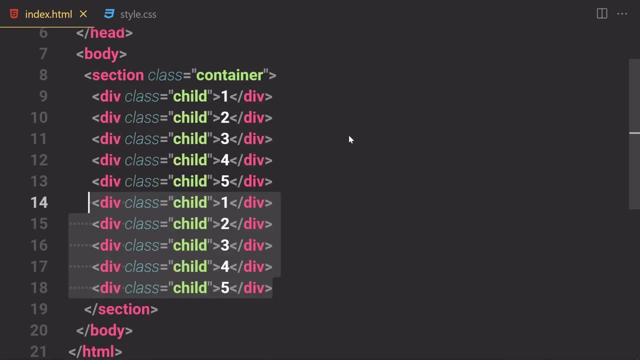 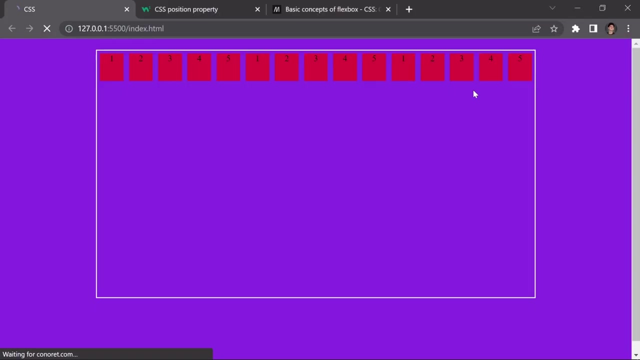 called a flex wrap property. so before we do that, we need a lot of content in here. so let's suppose if i just select that and if i duplicate the like one more time and save it, so we can work with a lot of contents, just like that. so now, here you can see. you know, i'm going to duplicate one more time. 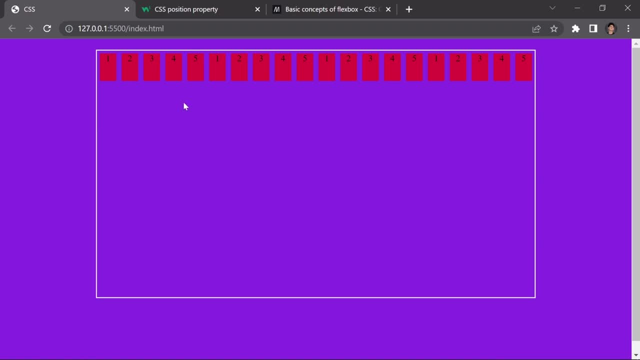 and now here you can see, and now here you can see. our children are now jamming together in each other right here and here. you can also see that with this change a bit. so if you want to push this item to the new line, so we can also do that. 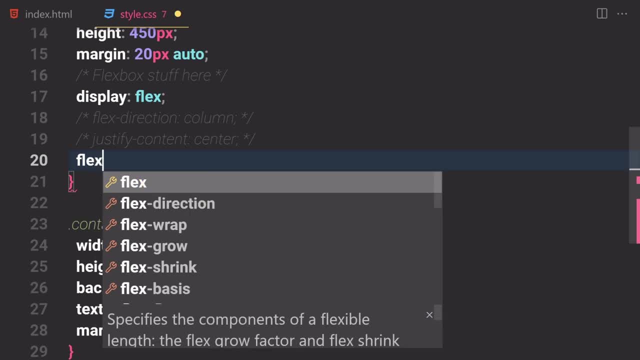 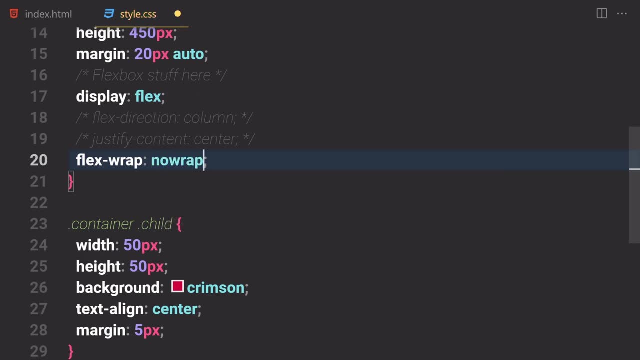 by using or awesome property which is called a flex- uh, not flex, yeah, flex, wrap of wrap. so by default the value will be set to no rep. so if you just write a display of flex to the default value, it will give us of no rep. so if you save that, so no wrapping right here. so in this case we want: 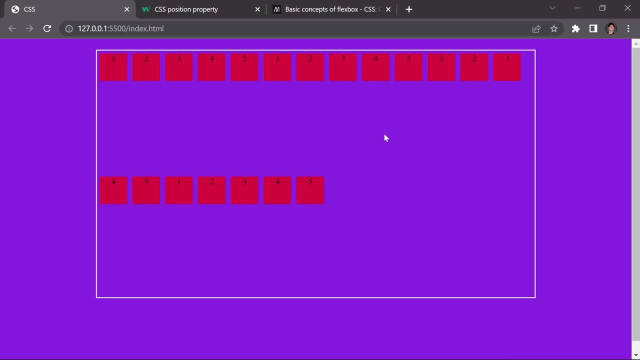 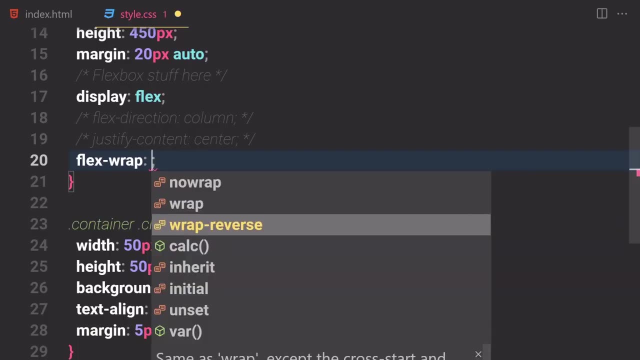 them to be wrapped, so we can just write as flex wrap to wrap. and if you save that, so it will not just wrap these items. so if you save that, so if you save that, so if you save that, so if you save them to the new line right here, okay, so that's that we have. we can also have a wrap reverse if 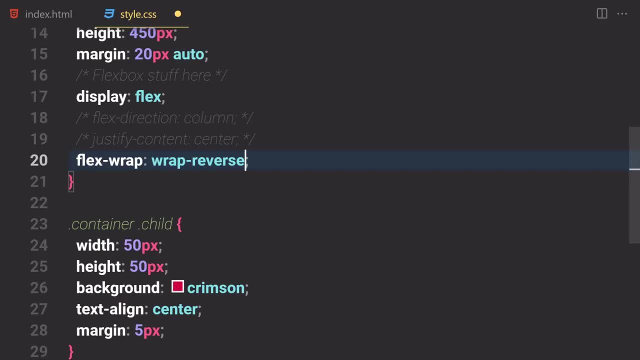 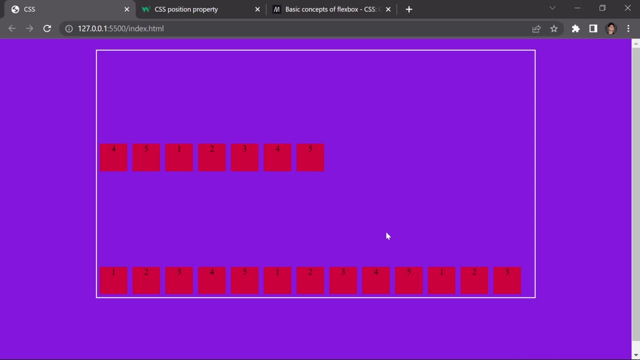 we want to, so we can reverse or wrap right here. so if you save that and boom, here you can see first of all we get four, five, and this is a random word, so that that's why we cannot see everything a bit clear now. you have to trust me that we can also do our rap reversing. 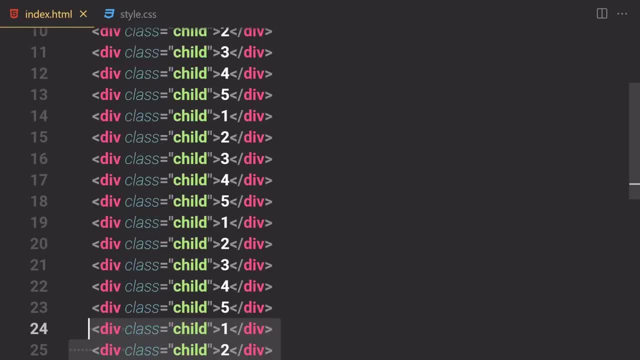 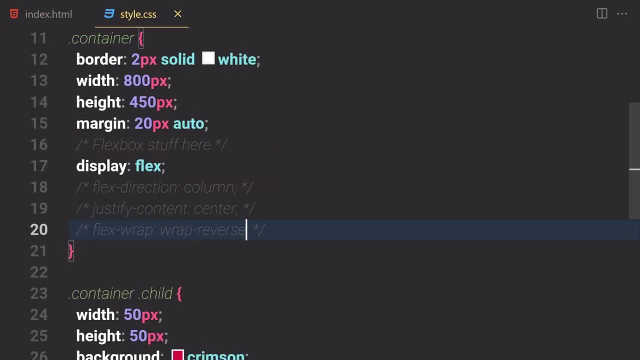 by using a flex wrap property. so i'm going to just comment this line out and i'm going to also undo this stuff. so if you save that, we get to this layout one more time. so that's it about a display: flex direction. justify content. i'm going to push this one to a. 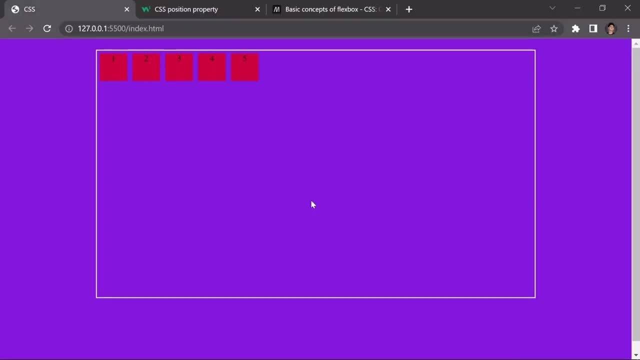 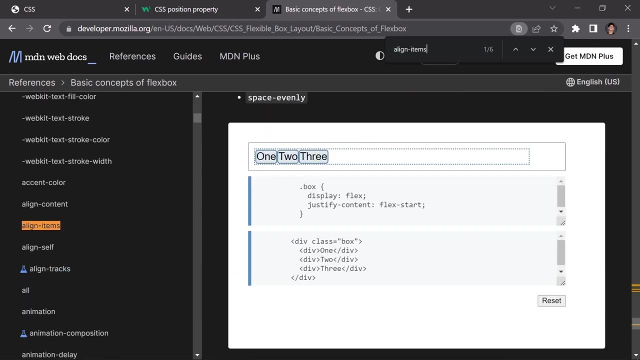 bit down. and now the next property which we are going to be learning about is align items. so this one work on a main axis and now, if you just search for, um, align items, okay, so let me just search for align items real quick. so here you can see, we have this align items property and the align items. 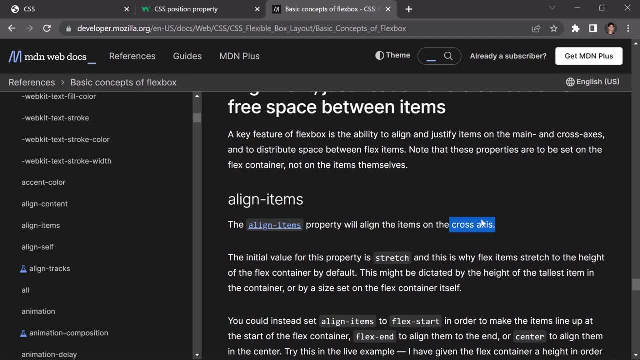 property will align the items on the cross axis. remember, justify content property will work on a main axis and now align items property will work on a cross axis. okay, so, uh, what do i have to do? i'm going to comment this out, or you know i'm going to. i'm not going to comment this one out. 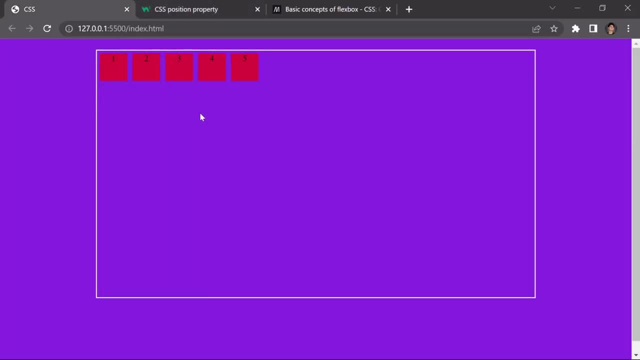 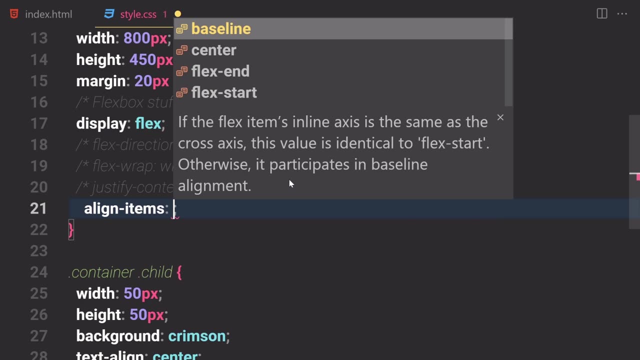 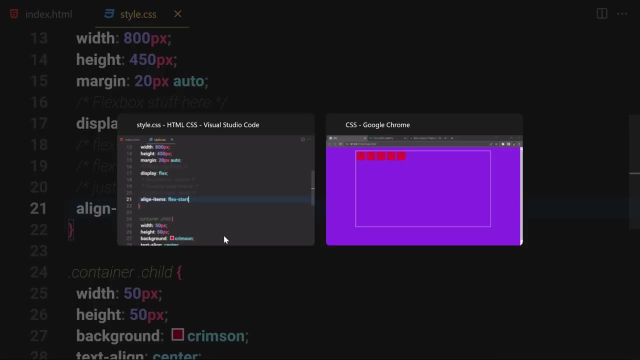 so by default we get this layout right here. so everything's- uh, i mean like justify content will be set to by default flex start. so now let's just work with or align items properties. so by default, if you just write like display flex, so by default it will give us the value of flex start. and if you 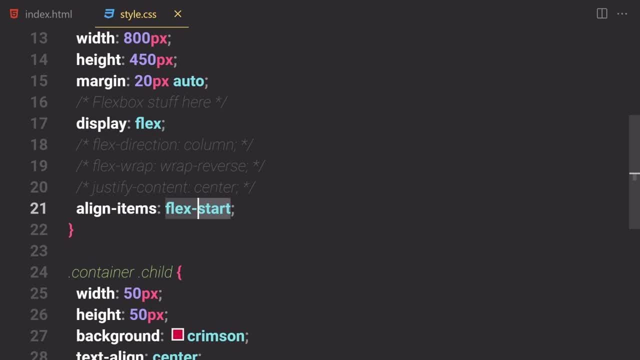 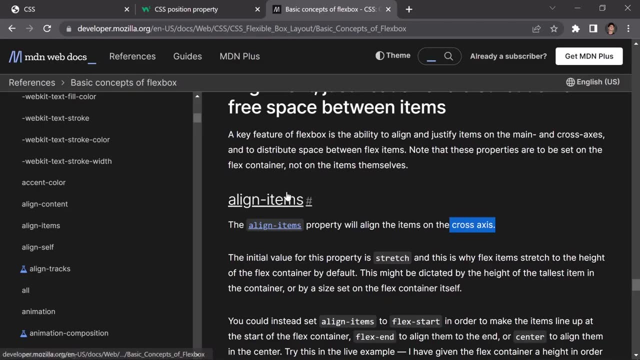 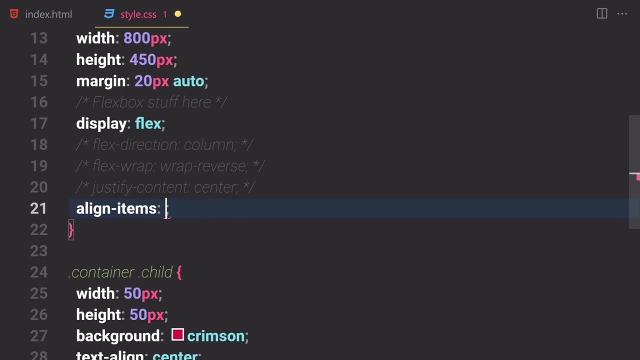 so nothing's going to happen right now. but we can also write a flex end if you want to. so if you save that and boom, it will push everything to the bottom right here. that's because align items- property- work on a cross axis. you just have to remember that we can also do centering. so if you just write like, let me just remove that. 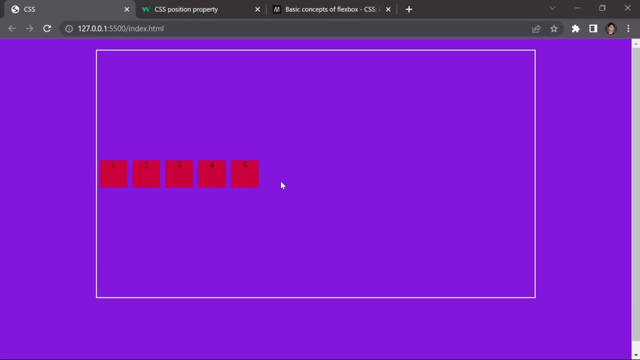 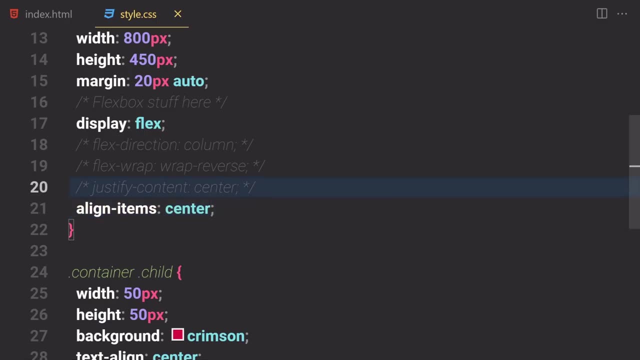 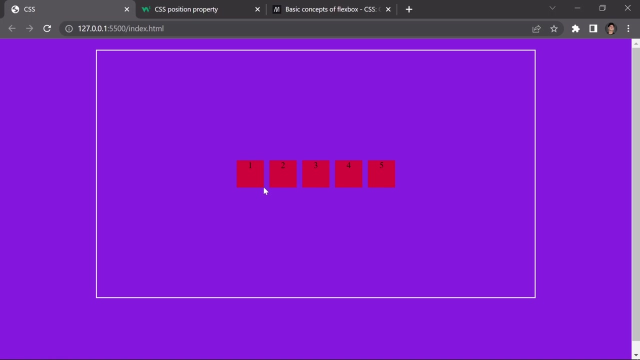 and we just write like center and if we save that and boom, it will be now perfectly center. so if you want to perfectly center this item right here, so for that we just have to uncomment this justify content property, and if we save that and boom, we now get totally perfectly center divs right here. okay, so these divs are now totally perfectly. 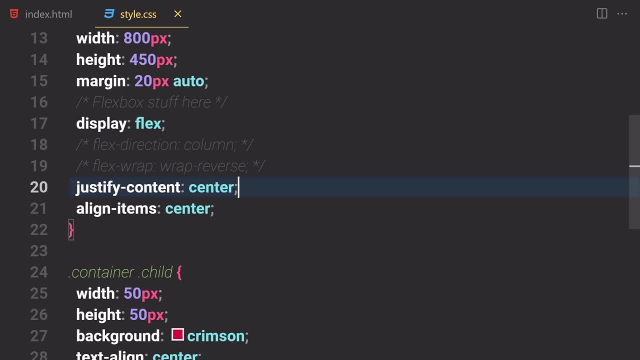 center to our viewport right now. so what do we have to do now? we learn about a justify content property, align items property. we can work with this. so by default, um, that's flex start. so let me just set that to like, first of all, flex, um, and maybe- and this one will be now set to center, or 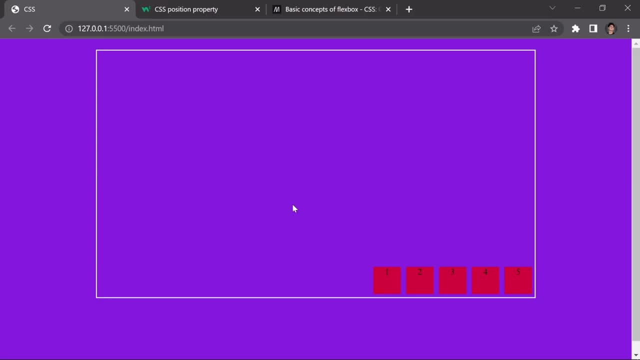 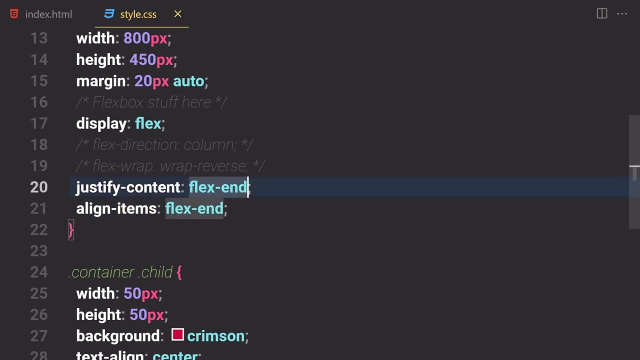 this one will be also set to flex, and so if you want to save that, so now just push it to this end here. so if you just set that to like a flex, start and you know what? that was just a default value for both of them. but let me just write like we already write: center, center. let me just write a. 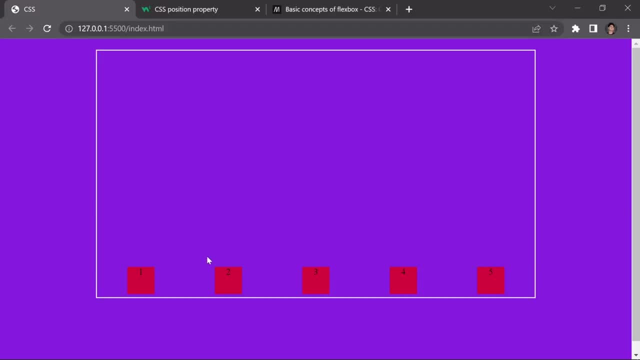 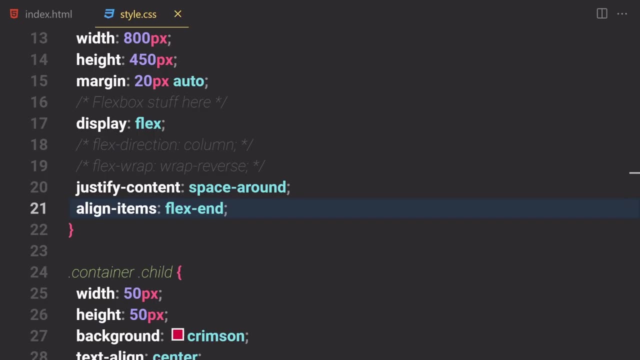 space around in here and this one will be flex end. and now, if you save that and here you can see it, unlock uses like a little bit of spacing right here and it will be at the, i mean like it will be at the bottom right here. we can also change this one to like flex start- flex start. 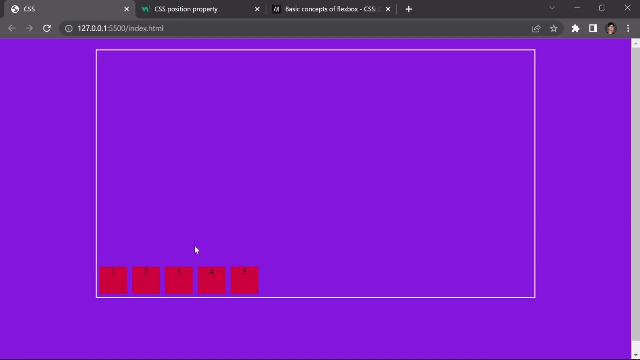 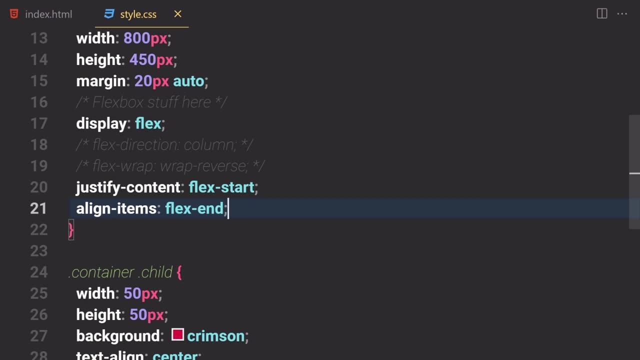 and the other one will be flex and if you save that and it will now push it, everything right so we can play around with that and i will highly encourage you to play around with these properties and values. i'm just showing you everything, but i cannot show you everything. you know like i cannot. 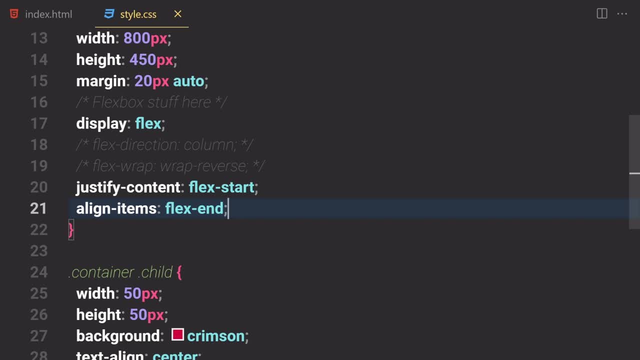 play around with all of the properties, because it will take a lot of time, it will take a countless hours to work with that. but i just kind of want to give you the test of everything and you have to figure out, like, how your layout will look like and how you should structure everything. so now 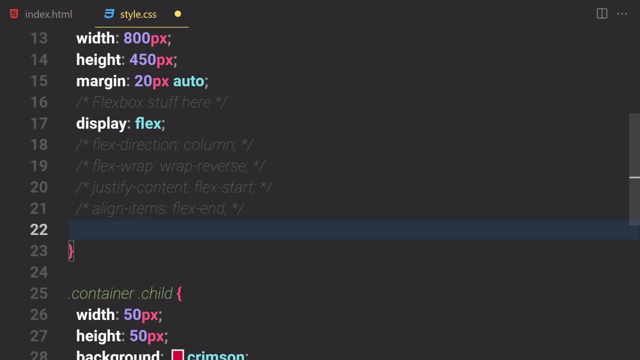 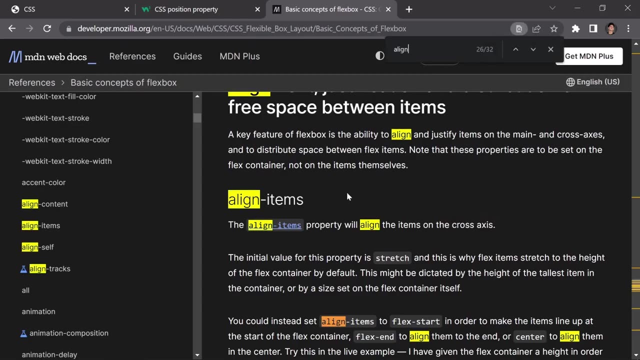 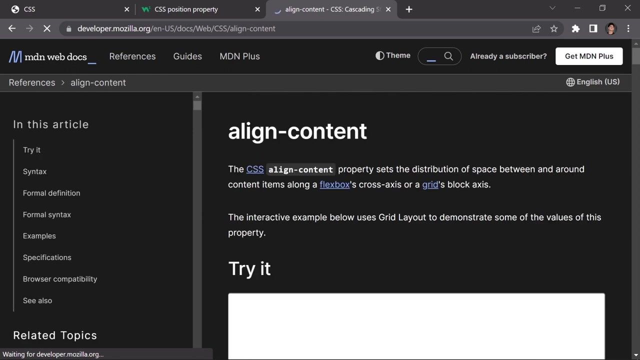 that we learn about align items and these stuff. now, the next property which we are going to be learning about is something called align content property. so let's just ask our good old friend: like align content. okay, so it will now ask us to go to this page, so i'm going to click on there. so it will now brings us to this page. 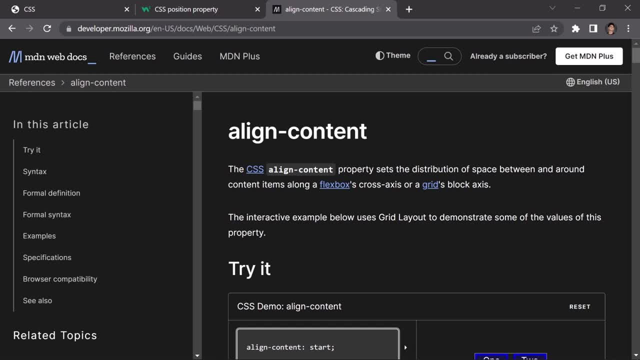 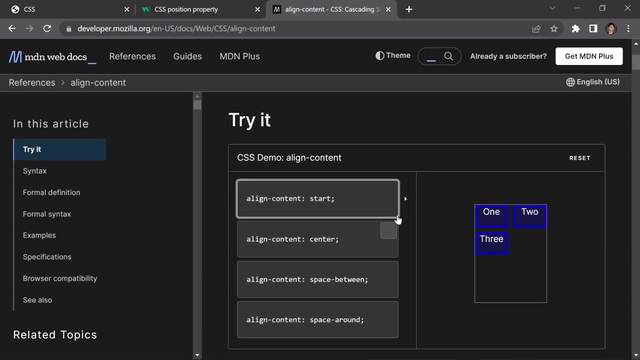 so the css align content property says the distribution of a space between and around content items along a flexbox cross axis or a grid block axis. so for that we are going to be need a few more divs. uh, okay, so i'm going to duplicate that a few times and now, if you save, 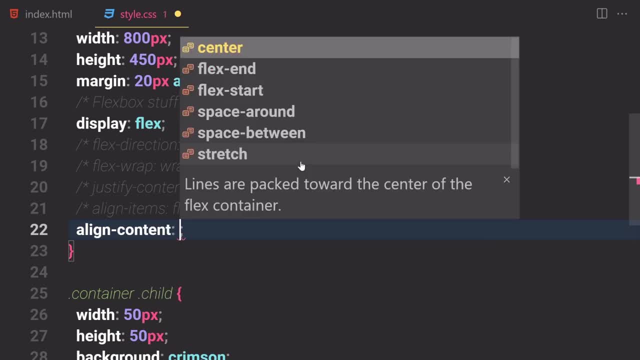 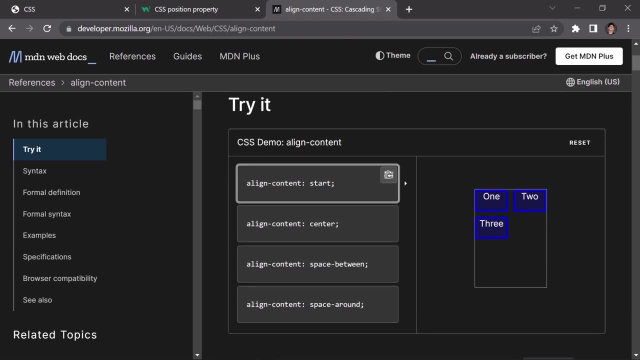 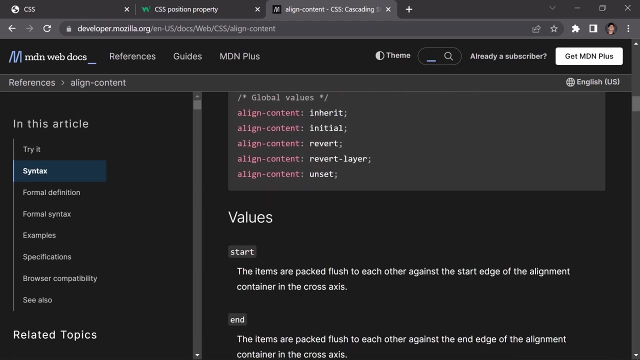 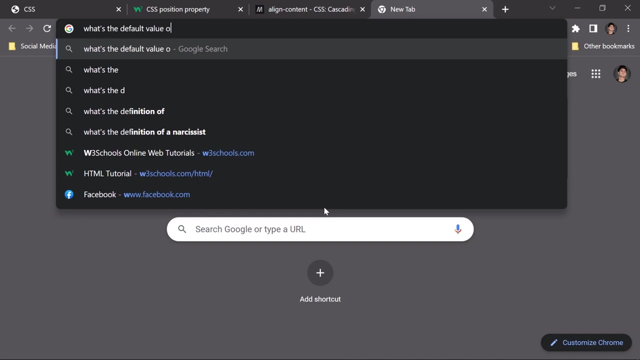 there and now here. we can just use like align of content, and now here, uh. and, by the way, what's the default value of align content? okay, align content. i guess the default is start. uh-huh, i guess the default is start, and we can play around with these if you want to. let me just ask a google like: what's the default value of? 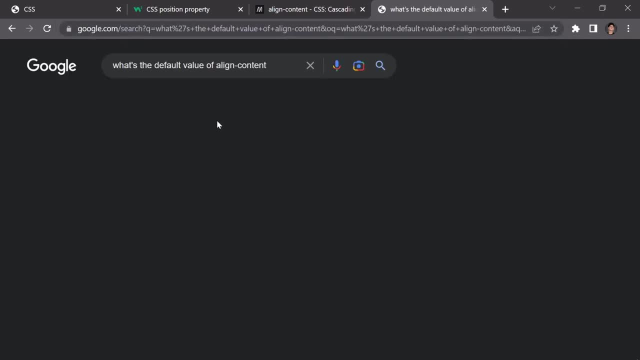 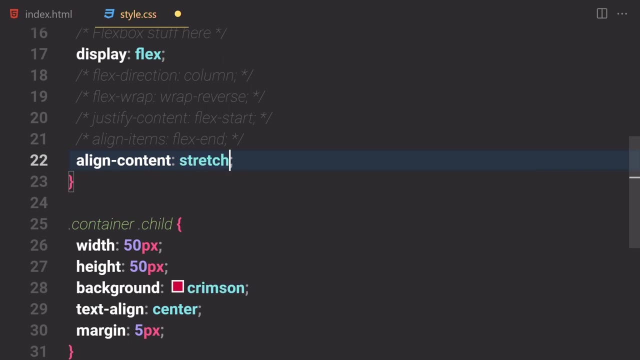 align content. so i guess: okay, so it's a stretch, it's not a flex start, it's not a stretch, it's not a uh stretch, so a stretch work like this. so if you just write a stretch, so it's a by default value and if you didn't provide any width and height to it, or you know, i'm going to just 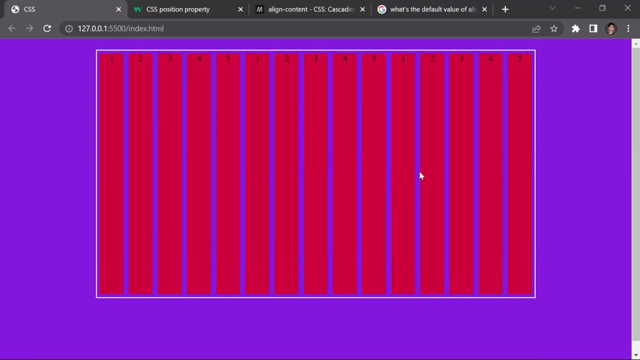 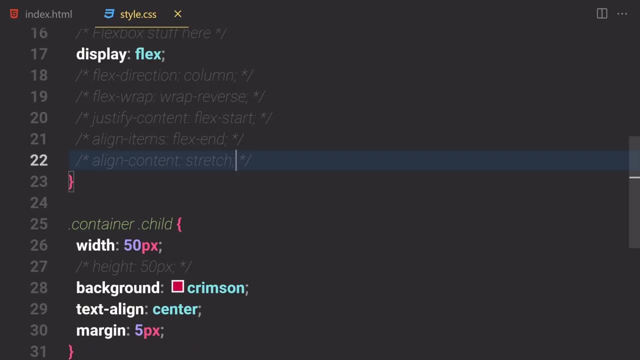 uh, comment out this height from now, and if you save that, and here you can see this is the stretch behavior right here. if you're uncommon, or if you comment this line out, and if you save that, so this is the default behavior. that's because we provide height to it, so that's why we are getting. 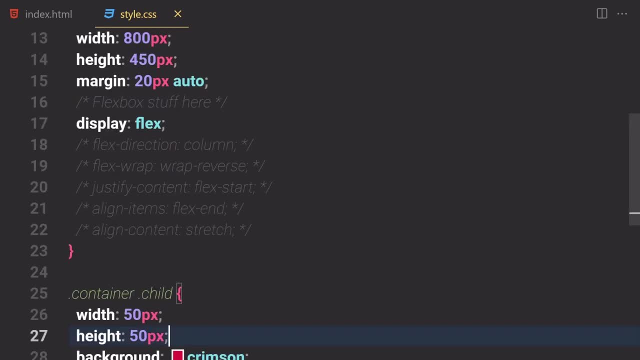 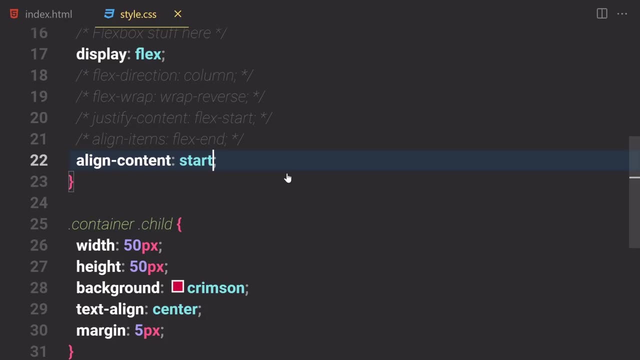 a height right here, okay, so you just also have to keep that in mind. and now let's just start with a working on a start. so if you just write a start- and this is going to be the start- we can also write an end: this is going to be the end. okay, it's not working. i don't know why we have a line. 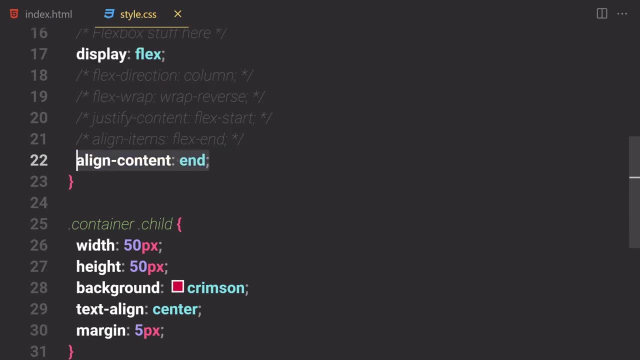 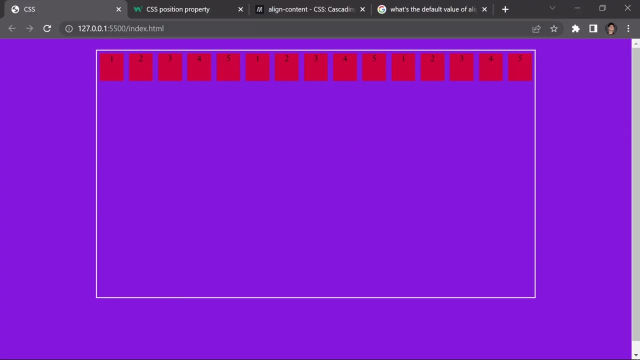 l-i-g-n, let me just write it one more time, l-i-g-n. and then we have content and let me just write a center maybe, uh, center, and if you save that, i know it's not working. okay, so we have to set or flex wrap to be wrapped, and if you save that, and now here you can see, it will center up. 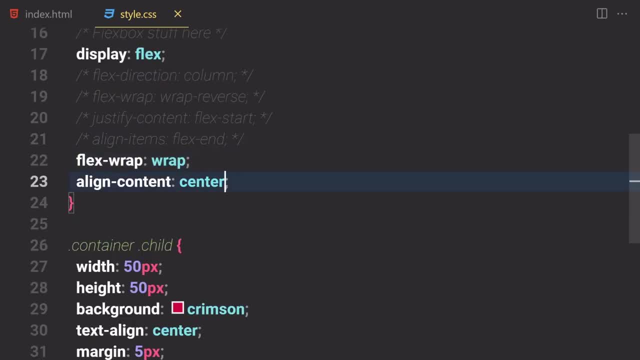 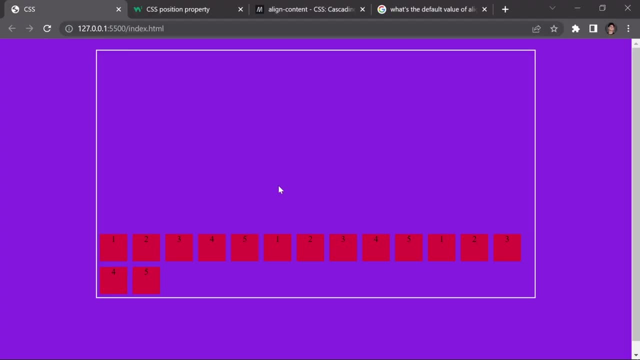 everything right here we have. use this flex wrap of wrap and now, if you want to go to the start, so we can use a start, we can go to the end if you want to, we can use a space around and it will not provide a spacing around the items and we can also use a space between. so if you save that and boom everything. 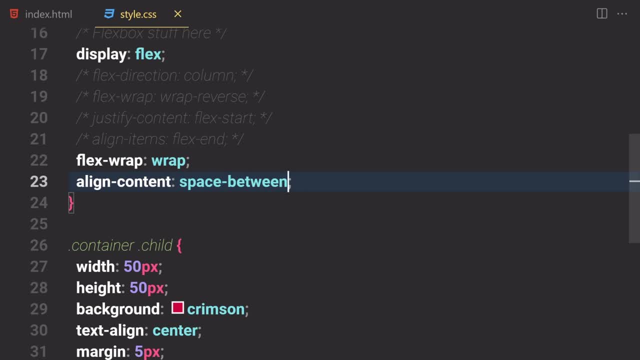 is working the way we expect to work. so i don't want to waste your time, uh, writing all of these properties in its values. so i'm going to just remove this flex wrap or, you know, i'm going to comment both of them out if you want to uncomment it. so you cannot uncomment just a single line. 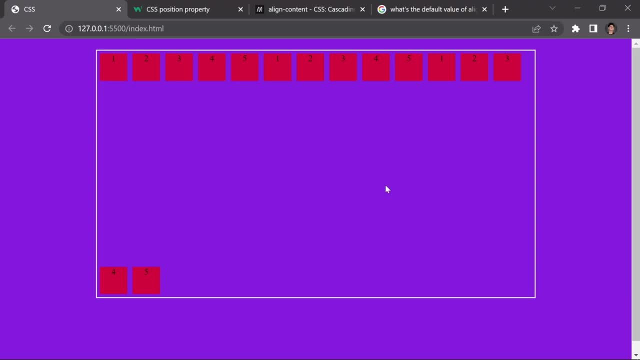 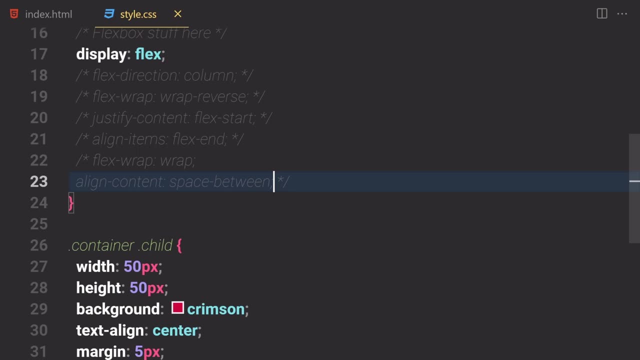 you have to uncomment both of them, and then you can save it, and then you can save it, and then you can save both of these lines at once, and if you save that, and then everything will work the way you expect them to work. okay, so now we cover half of the flex box. now it's time to work on a, just a. 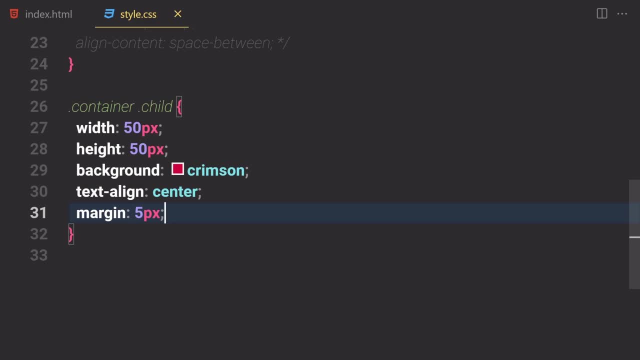 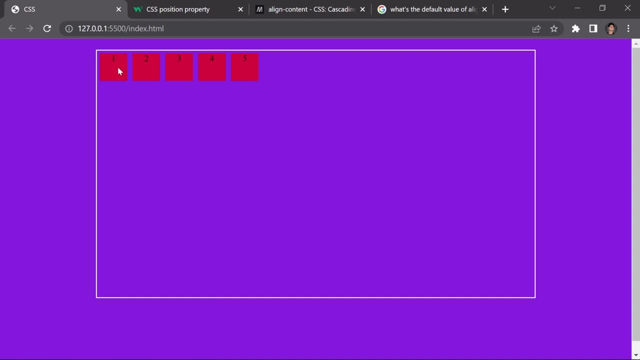 specific children. if you want to just move around one child at a time, so we can also do that. so first of all, let me just uncomment or undo this step. so if you save that, so here you can see, we just have like uh divs from one through five right here, and now you go towards css now instead of 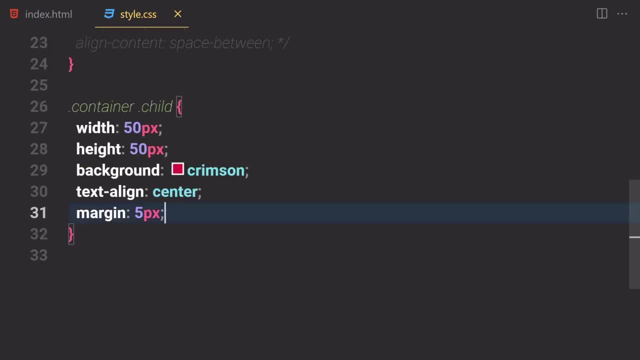 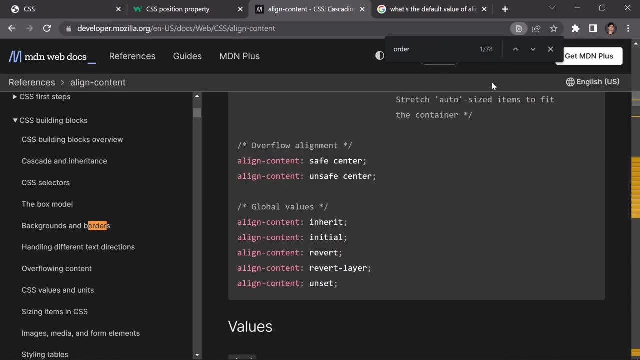 we can write it now inside a children, because we are working on just a single property. so now let's just ask our good old friend, like, what in the world is ordered? so if i just write an order right here, okay, so, okay, it gives us a lot of uh, oh, my goodness, these are a lot of order properties. so 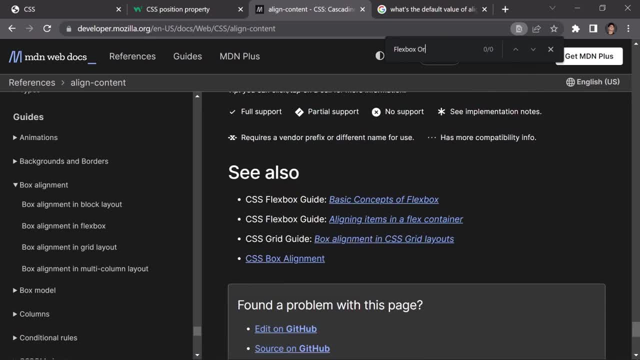 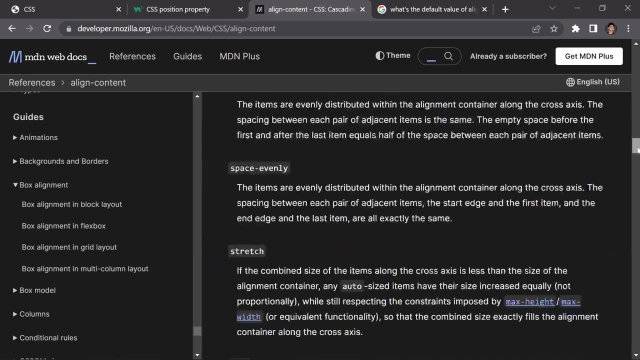 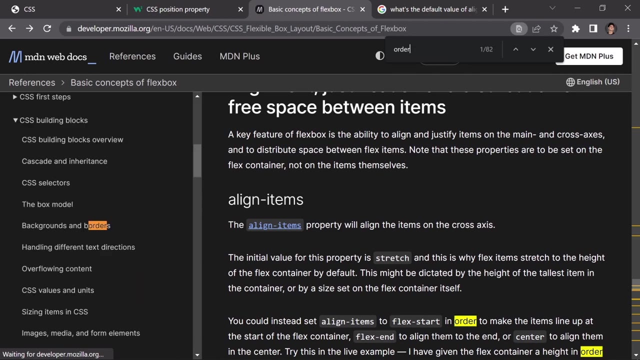 flexbox flexbox order, come on. okay, so we have to find that out anyways. so flexbox order- property is nothing more, but they will just provide a little bit of order to it. so i'm going to go back and now let me just see that order in here. okay, so we have order. okay, we got 82. uh-huh. 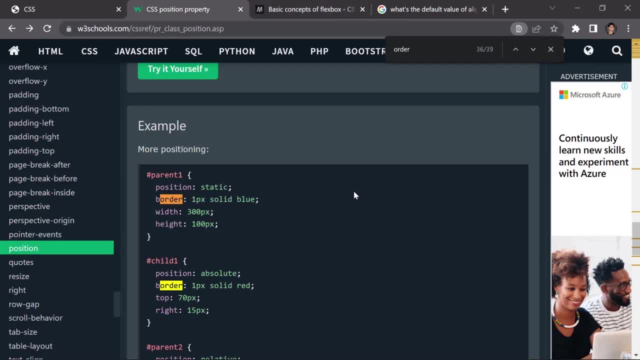 you know what? let me just ask from this friend: so order, property, flex order, or you know, let me just write a flex first of all. okay, css, nobody's helping me in this case. i guess i should have had to expand everything manually. but you know what? i'm gonna write a flex. 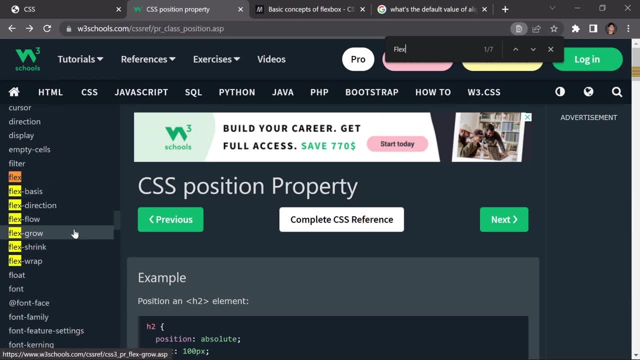 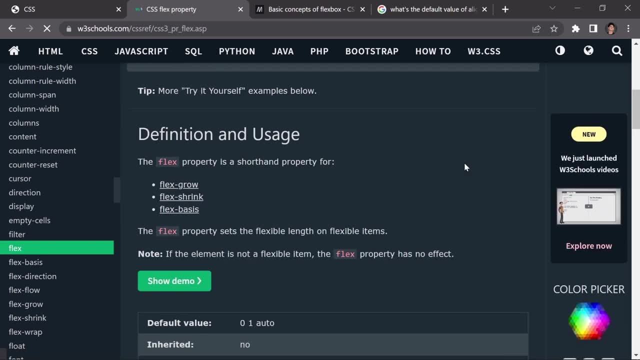 in here just like that. so we have flex basis, flex trap, shrink grow flow and stuff like that. i'm going to click on the flex one so i can go to the flex box right here, and i'm going to have to search for order right now. so order- uh, we got a borders and 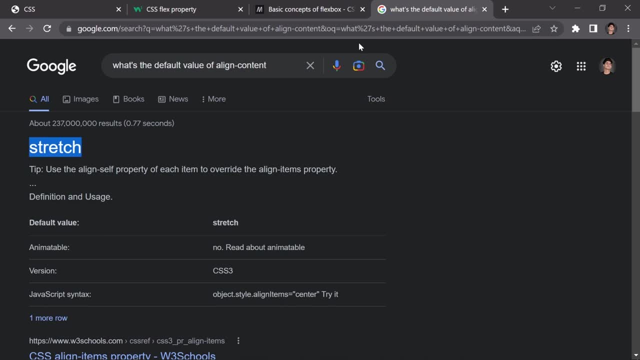 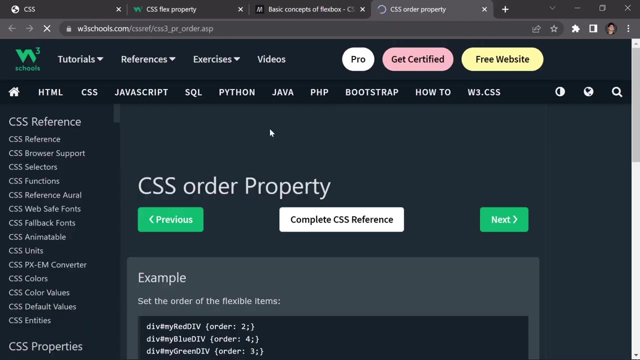 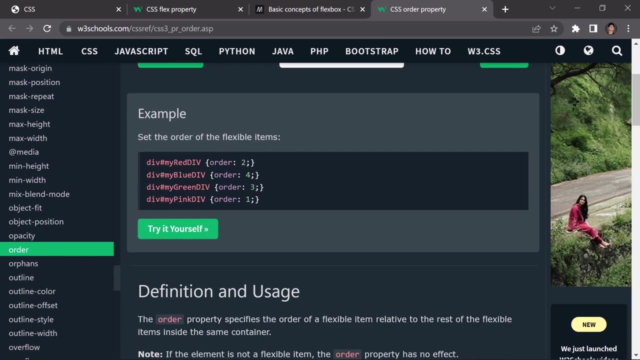 we don't have any order. let's just ask our friend google um flex box order property proprty. all right, so it will. now brings us to this w3 school. okay, i knew there is something inside this. uh, i don't know. it wasn't helping us at first place, so set the order of the flex item to be like some order. 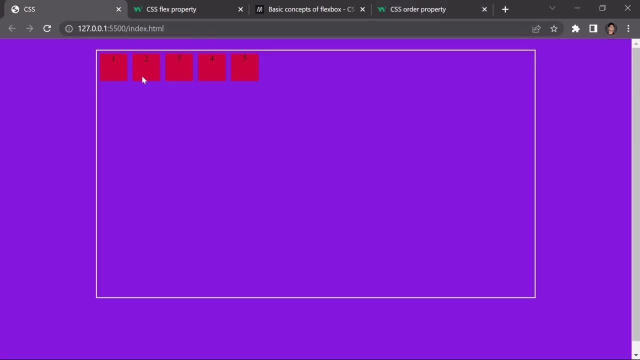 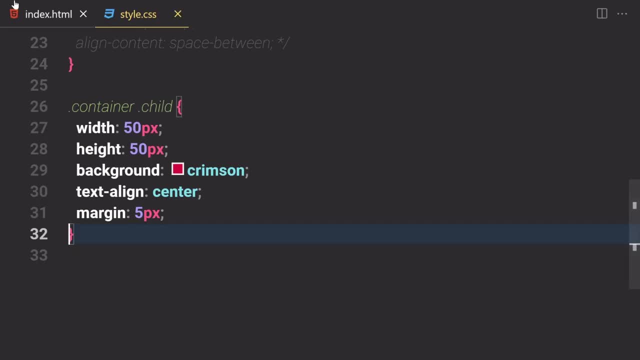 one will be zero and also this one will be also zero. okay, so i'm going to select just one child, like maybe this third one, and i'm going to just provide like a special class to it. so i'm going to just save that and now i'll just select this special class. so i'm going to just write like: 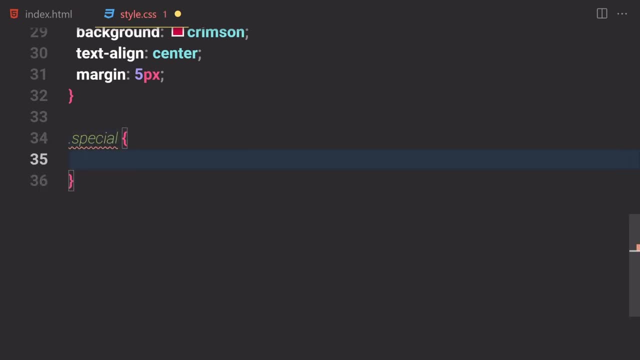 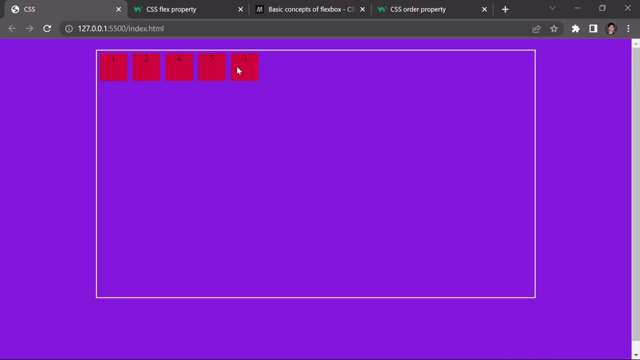 special, special. so now here, what do i have to do? i'm going to just write an order of one to it and now, if you save that- and now here you can see, it will now push it to the bottom right here, because all of them have the class of zero. now, this one is special and we 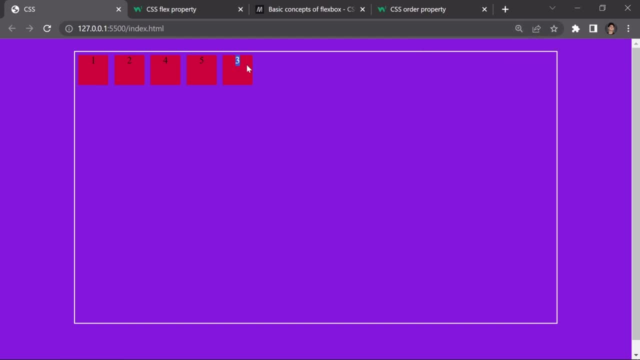 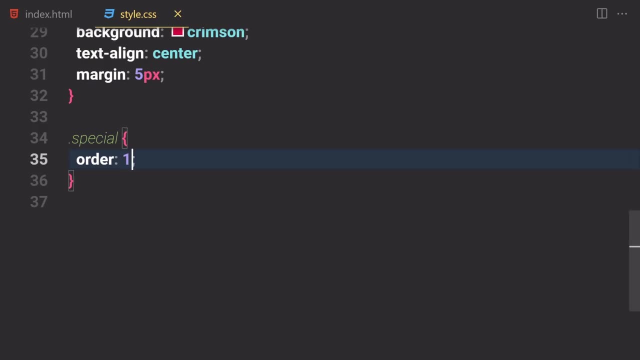 get the class of zero, and we get the class of zero, and we get the class of zero and we get the this one, the class of, i mean like the order of one. so this one is now special, so it will now push it to the bottom, and this is how you can reorder your layout: by using just an order property and 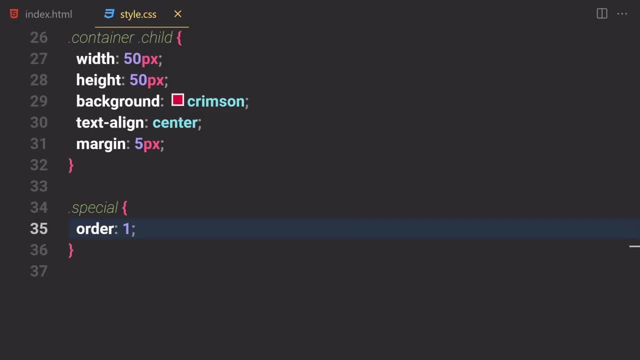 this is very powerful. so now, let's suppose, if you want to set this one to like order two, so for there we can just write like, i don't know, special two, and now, if you save that, and this is how you can use the order of your element, so i'm going to just write like a special and then two, and i'm 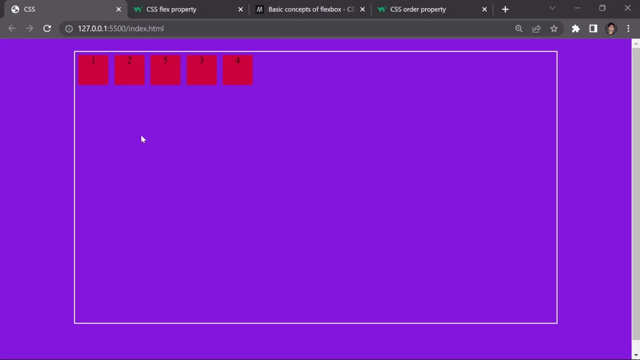 going to just provide like an order of two to this one. so now, if you save that, so what do we get? we get like one, two, five and three and four. this one has the order property of two. so this one have a high specificity. this one is a. 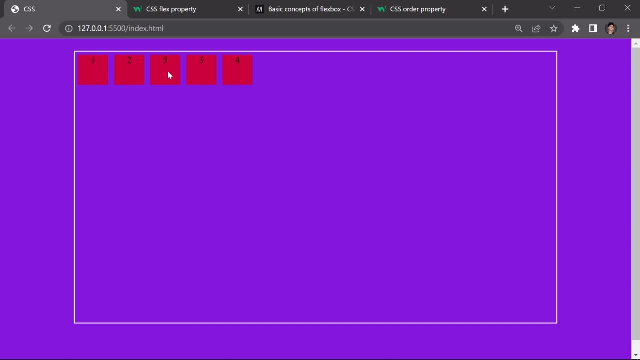 little bit lower than this one, and all of these have like zero one, so there will be a first, second and third, and you can also go with a flex direction of colon, so it will give you the same result. okay, so this is how we can work with a flexbox order property, but i just kind of want to show you is 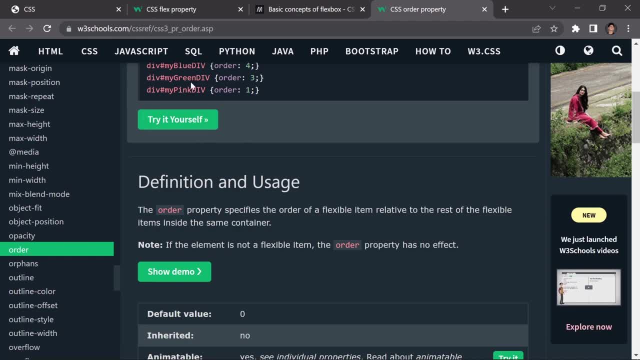 like where you would find all of these order and these order properties. so this is how we can work with a flexbox order property but i just kind of want to show you is kind of a single element properties and stuff like that. so that's why i 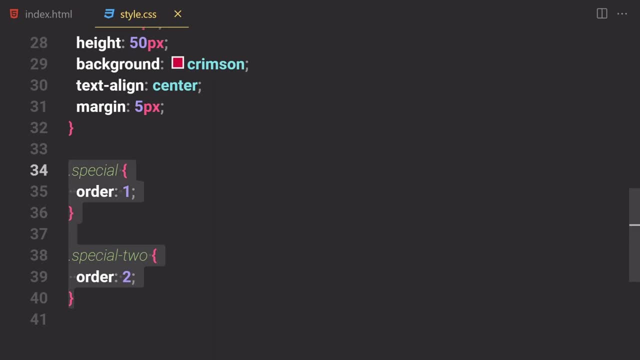 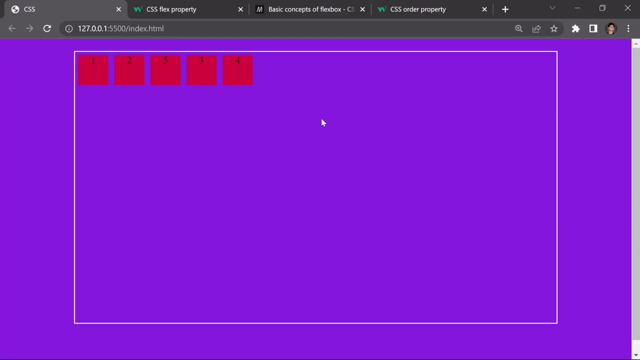 want to show you, okay, so what do we have to do? that we have to remove, or you know what? we are not going to be removing that, we are going to be learning about the next property, which is align self. so align self, as the name suggests. there, we'll just align that item to itself. so if you just write, 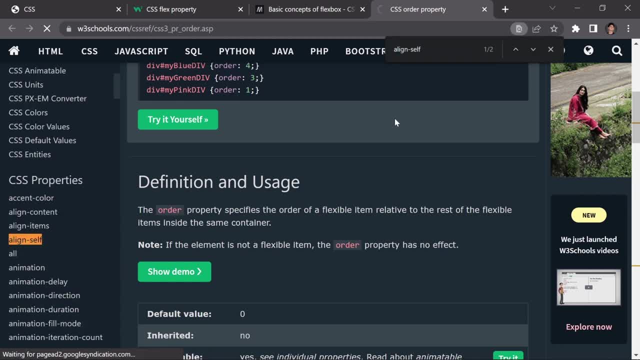 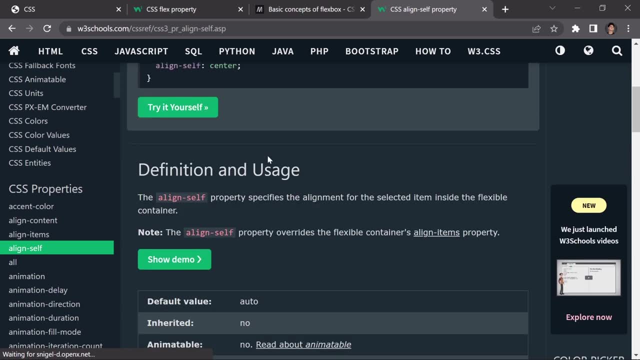 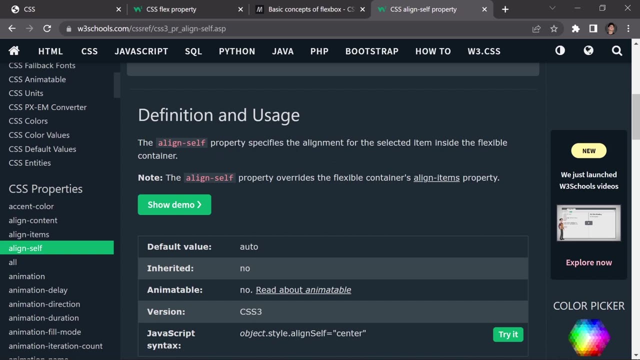 like align self in here and we can just click on that. and now here you can see, center the alignment of the one element of time inside of flexbox element. okay, so we can just work with one uh children of the flexbox by using align self properties, so the online self property specify. 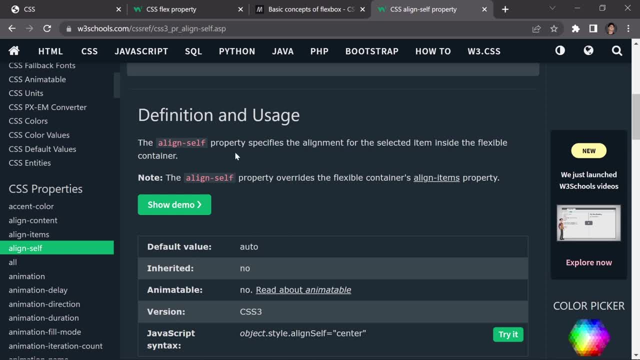 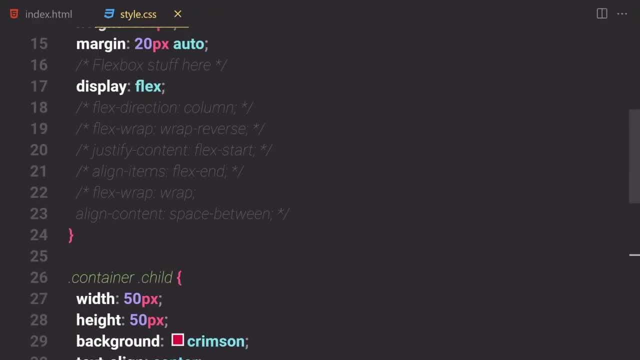 the align alignment of the selected item inside that flexible container. note that align self property. all right, the flexible container. okay. so if you have some um style inside this flexbox container, so it will override it, okay. so now we just give them a class of special to this. third, 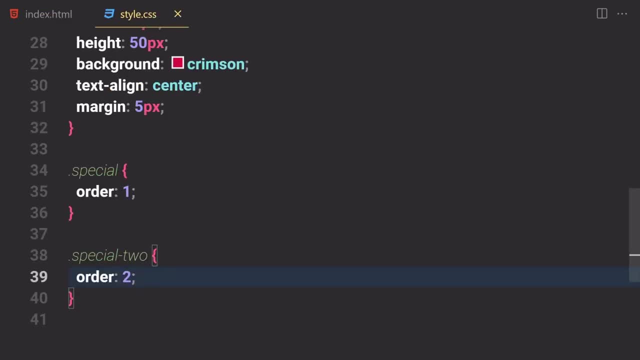 one and we want to make that to like center maybe, so we can do that. so i'm going to just remove this order one, i'm going to also remove this order property from there, and what we have to do. i'm going to just write like: um, not flex cell, but align self property and 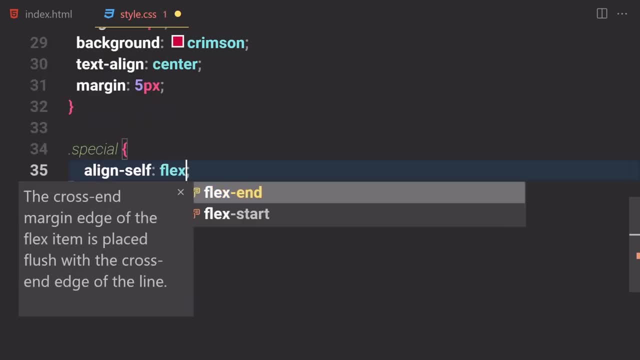 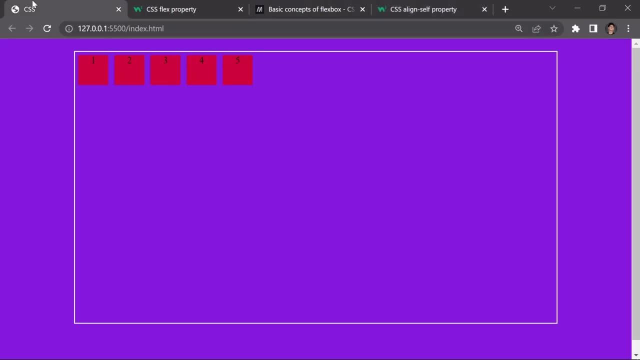 now, here you can see, we have access to all of that values, like we have flex start, we have flex and center and all of them. so i'm going to just write flex start and if you save that, if you go towards css, so it will be by default start like this one is special one. okay, so now we can use a flex start. 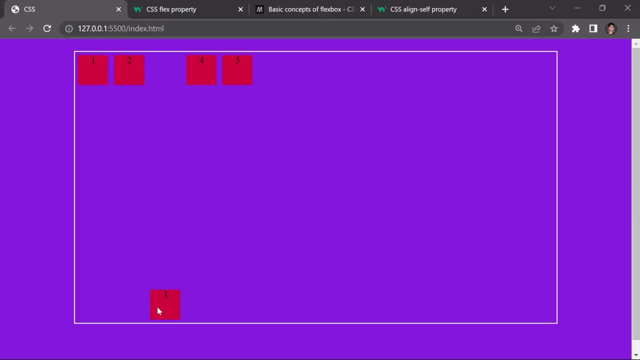 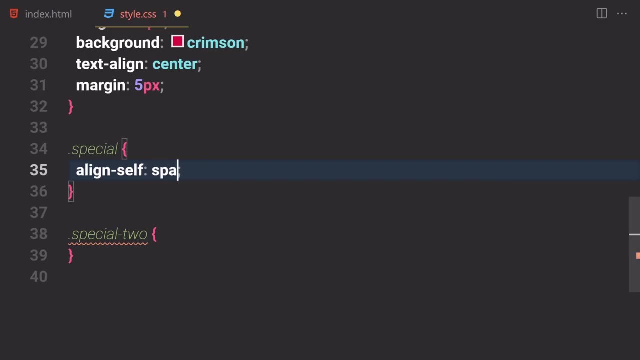 we can also use flex end and if you save that, so we'll now push it to the android here. we can also center if you want to. we can just use like center. it will not push it right here and we don't have access to that space between or space around, because we are just working on. 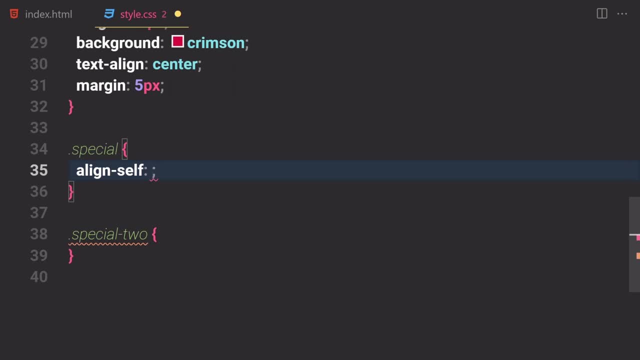 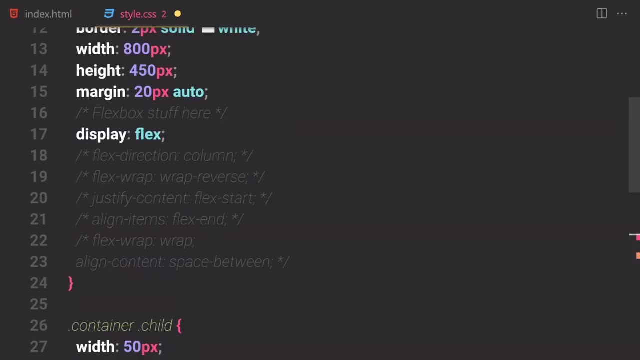 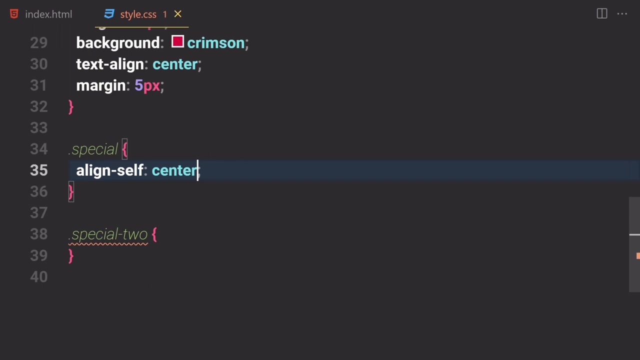 one single item. i mean like this: align self property allows us to just work on a one single property, but for that we have to select or item manually. and that container should be a display of flex. okay, don't forget that. okay, so we can just write like center in here and save that and it's now center this. so this is align self property and we 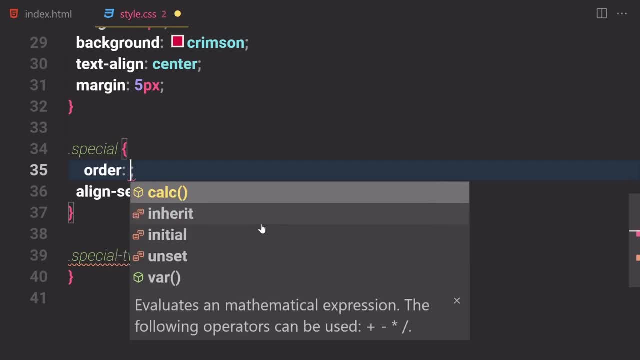 learn about order property. so you know, i'm going to just write like order of one in here. i'm going to comment that out so that we can forget that. so now we learn about a line itself. now the next thing which we are going to be learning is like, first of all, just save that, and this is how. 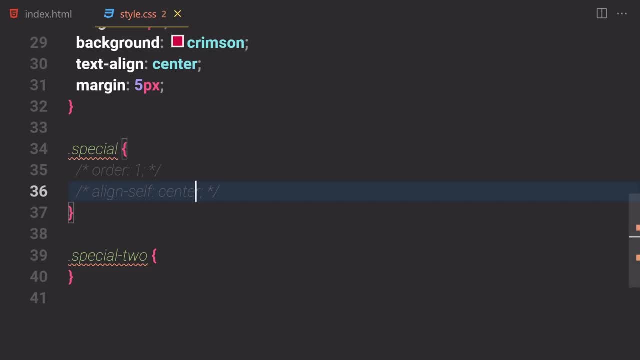 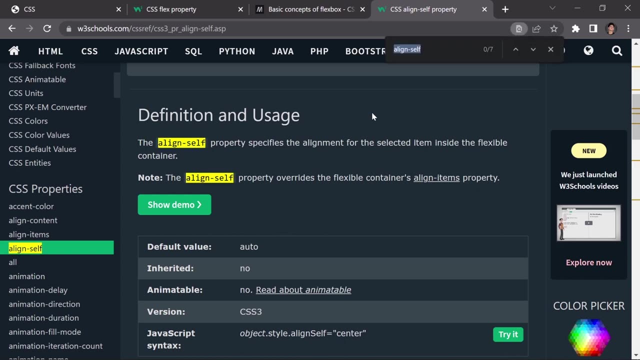 currently things looks like, and now the next property which i want to show you in flex box is something called a flex grow property, and it allows us to just grow one single item. so i'm going to just search for that like a line- not line, but flex grow- and if you click on this one, 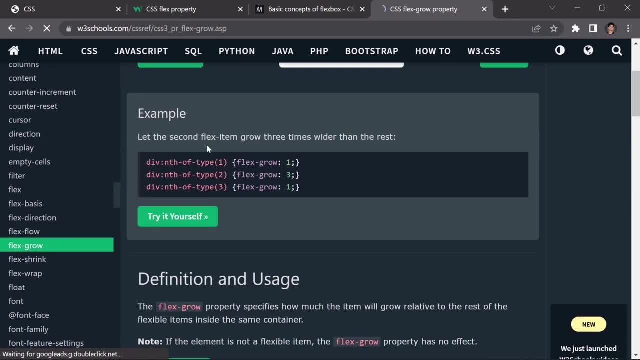 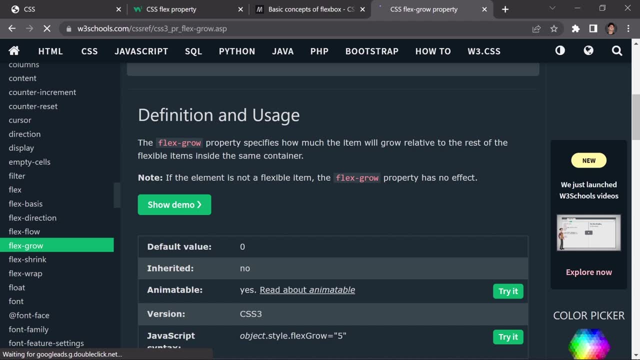 so it will. now brings us to this web page, right here, that the second flex. okay, that's not cool. so the flex grow property specify how much the item will grow relative to a reset of the flex item or flexible item inside that same container. note: if the element is not flexible item, the flex 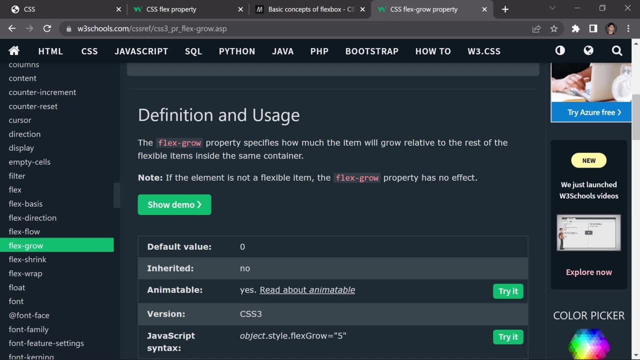 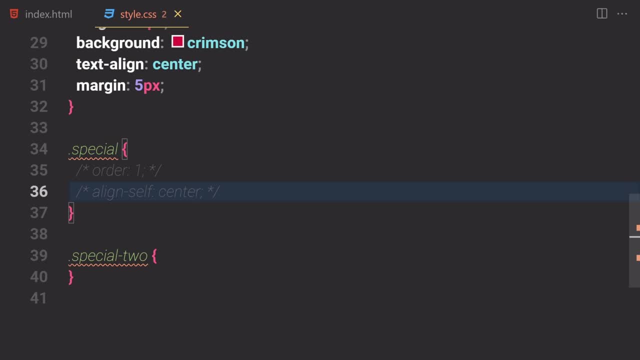 grow property has no effect on that. okay, so you just have to remember that in your mind. so now let's get into it. let's suppose we want to like grow this special class. so we want to like suppose, grow this one, so for that we can just use like flex grow property and we can provide like 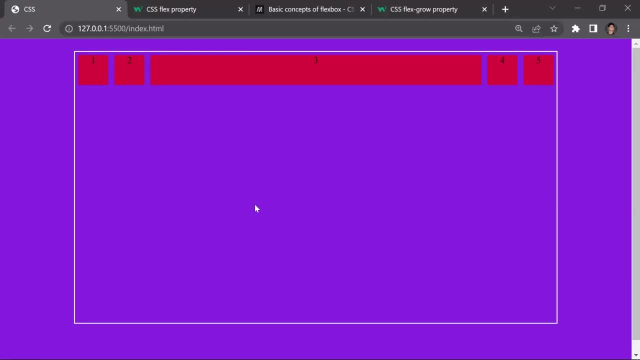 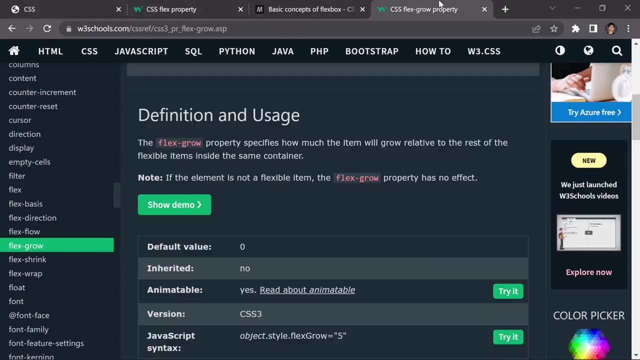 different kind of um, maybe two, and if you save that, so here you can see, it will now grow right here. so i guess the default value is zero for all of them as well. so now let's just ask from him: like, what's the default? okay, the default value is set to zero, as i said, so default value will be set. so 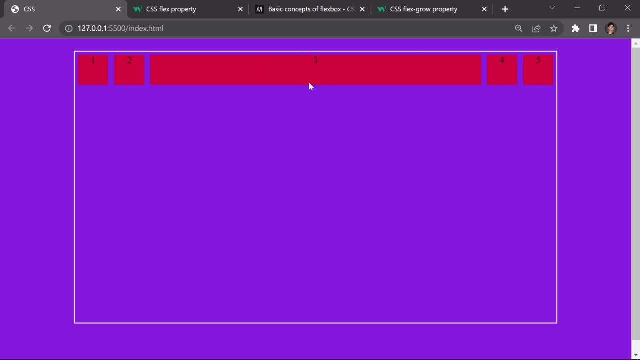 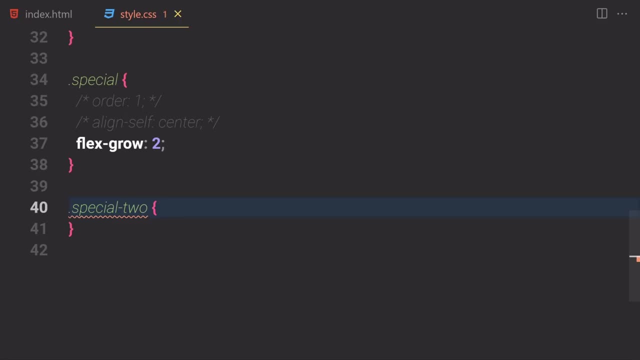 like these will have the default value of zero, and now we provide a one to it, so it will now take its entire space right here. okay, so let's suppose if you just select this special two and we just provide a flex grow property on it and now let's just use like 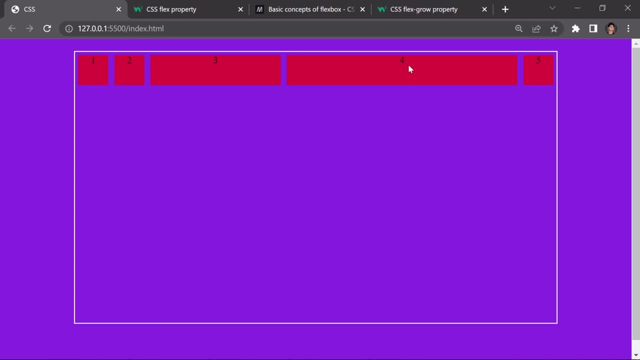 maybe four. and now, if you save that, and here you can see, this one will grow more than this one right here, and we can also change that one severed and boom. this is how you can grow and shrink your item- and, by the way, i didn't show you a shrink property, but this is how you can grow your items if you want. 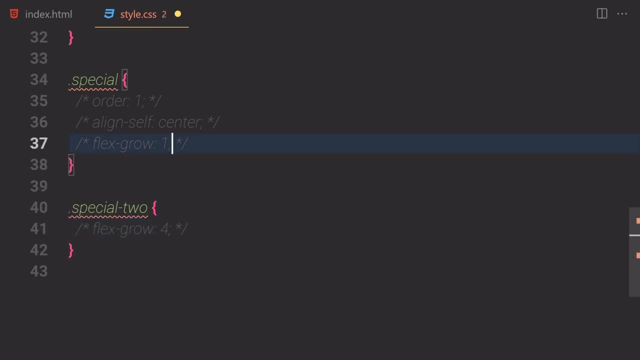 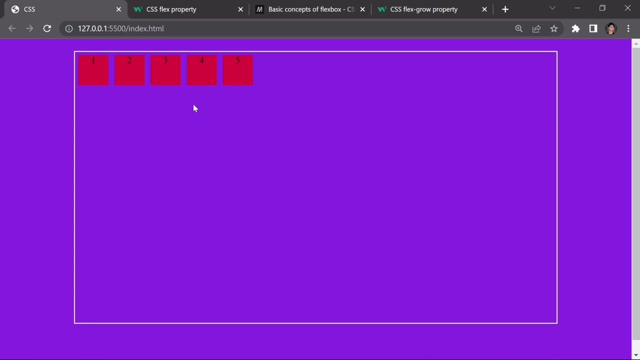 to. so now i'm going to comment this line out. i'm going to also comment this line out, and if you save that, and this is how everything's look like. so now let me just show you two more properties and then we are going to be totally done. 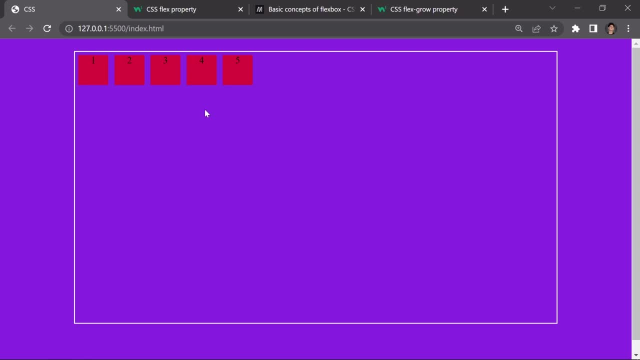 by flexbox, and then we can jump into the game, and then we are going to be playing a game. so what's the next property? the next property is something called flex and bases, and now let's just search for that. i'm going to show you the documentation of our flex bases, and, if you 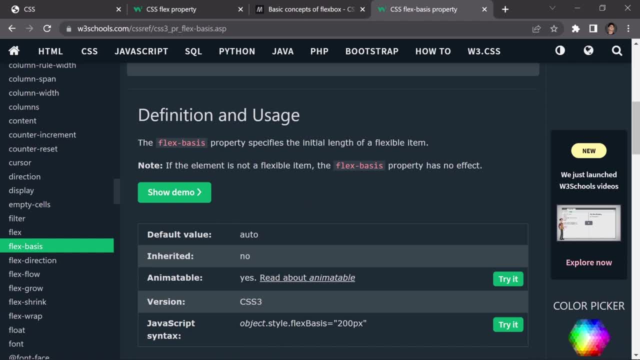 click on that, so it's kind of a weird one. so the flex basis property specify the initial length of the flexible item. note: if the element is not flexible item, so that flex property will be a have no effect on that and the default value will be set to auto. right here and now, let's just work. 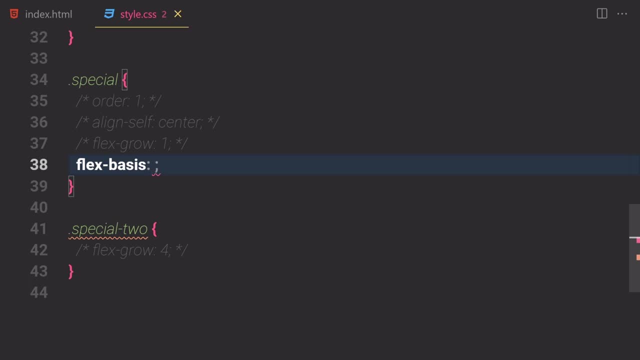 with that. so now, here we are going to be just specifying like, uh, i don't know, maybe i'm going to just provide like 20 pixel, and if you save that, and now here you can see, we'll now just shrink down a bit and we can just provide that like i don't know, flex bases, uh, of maybe four or you know. 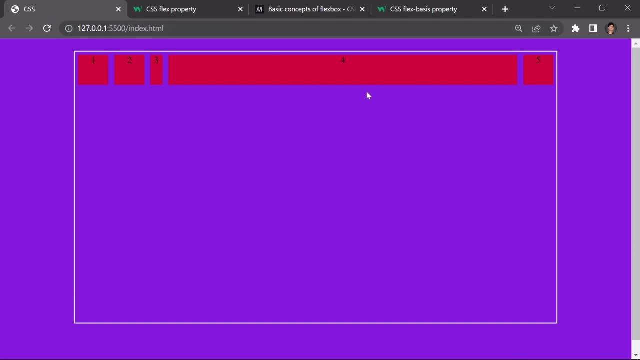 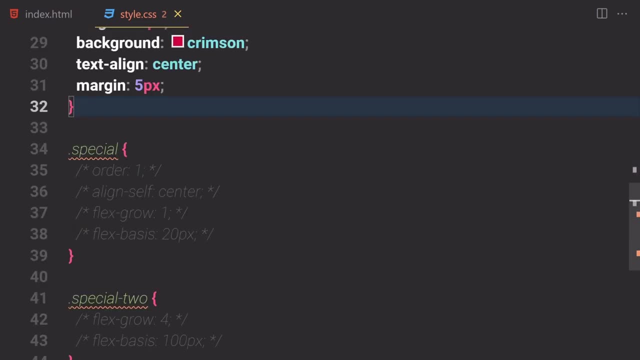 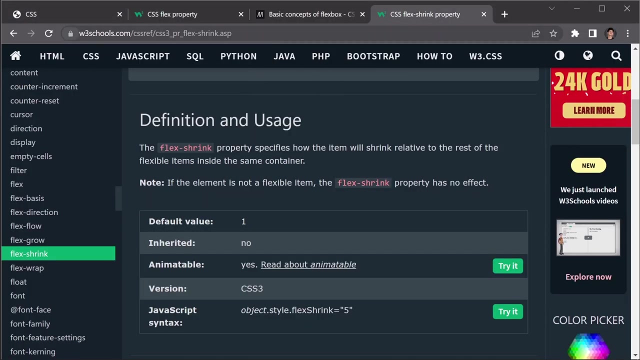 100 pixel to be fine if you save that, okay. so this is how you can work with the flex basis. so now the next property which i want to show you is called a flex shrink property. so i'm going to just write like a flex shrink right here, and if you just ask for google, like what is not google? but if you ask 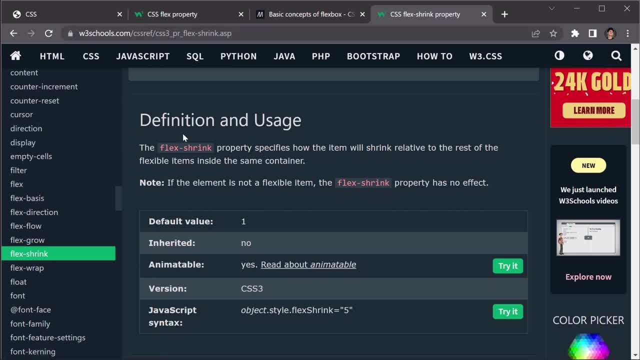 w3 school. like what is the flexuring property? as the name suggests, there it will allow us to shrink or item. so the flexuring property specify how the item will shrink. relative to the reset of the flexible item inside the same container. note: if the element is not a flexible item. 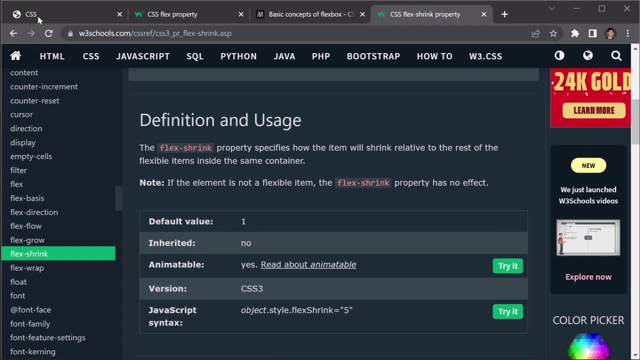 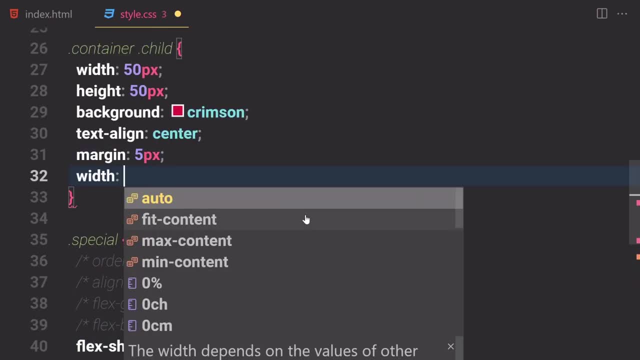 the flexuring property will not have effect on that and the default value will be set to one. if you want to work with the flex string property, first of all we have to provide a little bit of width to the item uh to the child. so maybe i'm going to just provide like 400 uh height to it. 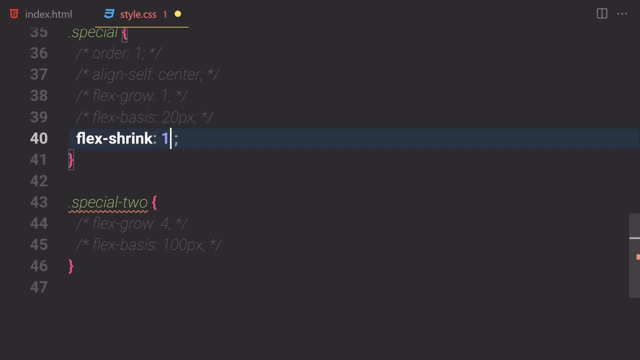 i mean like width to it. and now what do we have to do? and so the default value was one, so we can just provide two if you save that. okay. so here you can see what item will now shrink to that much. so if you just write one, this is the default behavior- we have a four or item will look like: 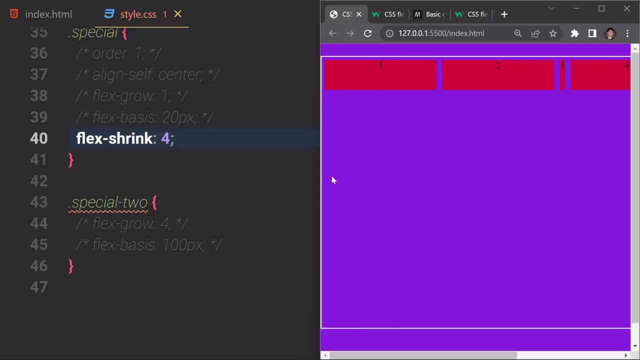 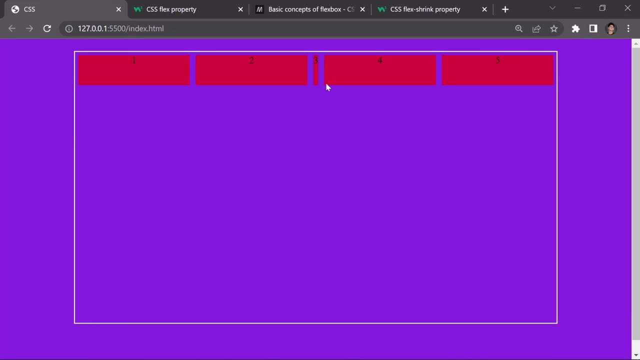 that. so now let's just write four and it will now shrink it like that much. okay, so we can just make screen size a bit bigger or smaller. so this is how the flex shrink property will work, so it will just allows us to uh, shrink down or element right here, okay, and we can just 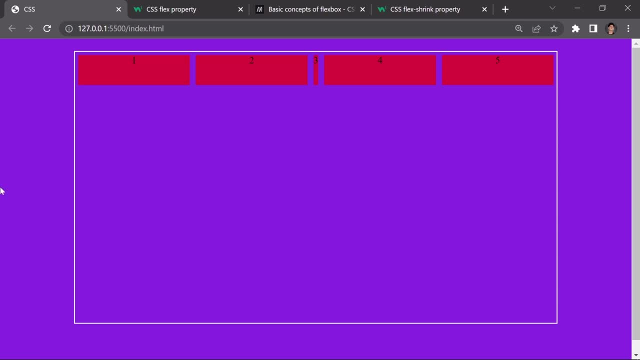 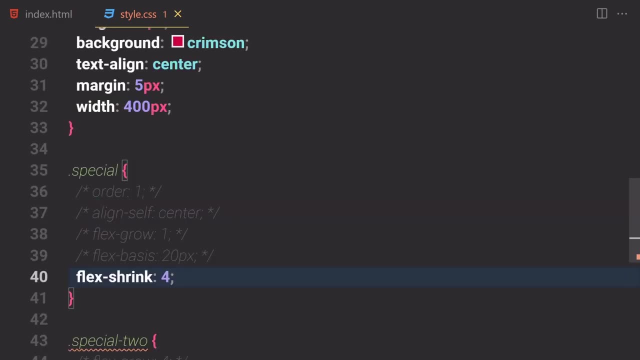 increase the height, i mean like the width, if we want to like 600 pixel. so, as the name suggests that it will just shrink out or element like, like flexuring property will just do that for us. okay, so now we are totally done with the flexbox. so we learned enough about flexbox, like we learned. 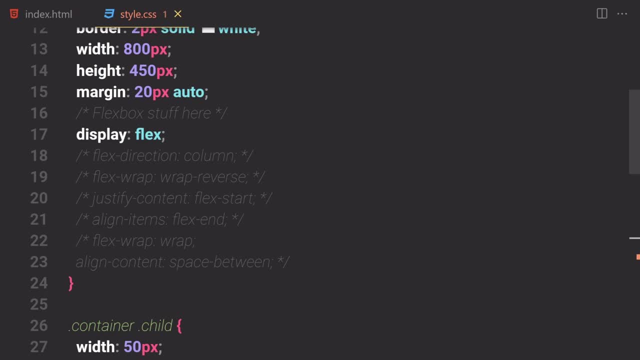 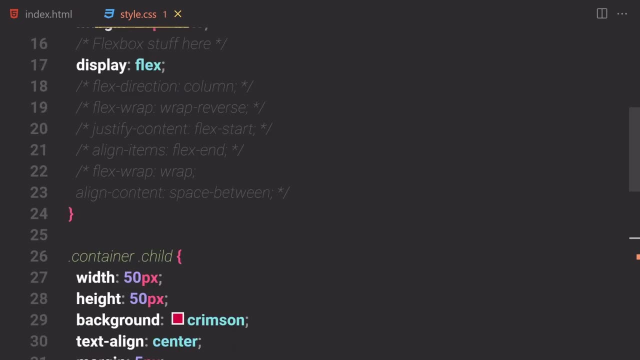 about a display property. we learned about the main axis and cross axis. learn about a flex direction property, which allows us to change the direction. then we learn about a flexbox wrap property and it will allow us to wrap the item, then justify content, align items, flex uh. 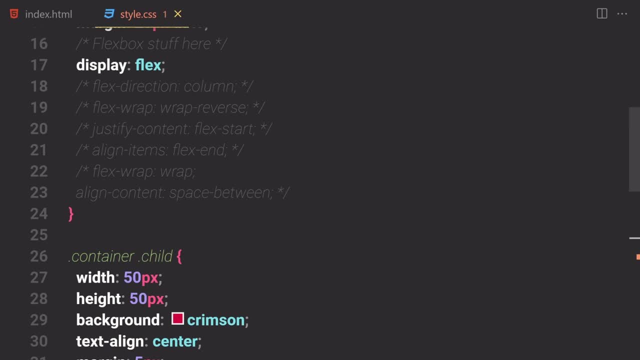 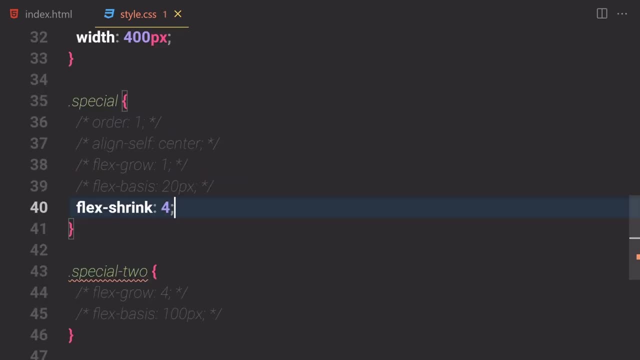 wrap. we learn that again. and we don't learn that, but we use that again. and then we learn about align content property and then we learn about how we can layout just a single item by using a order property and then align self flex, grow flex, basis and finally, we just learn about a flex. 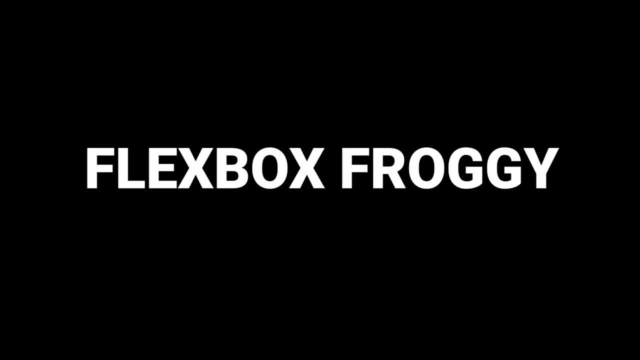 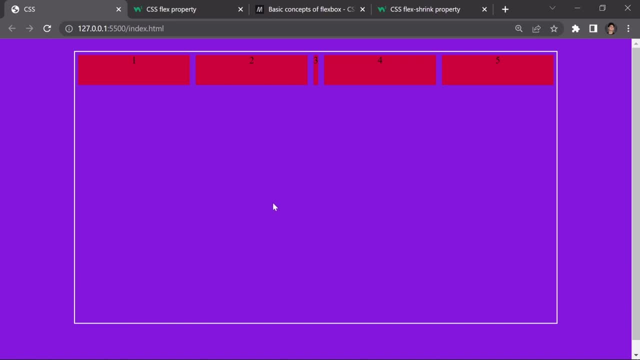 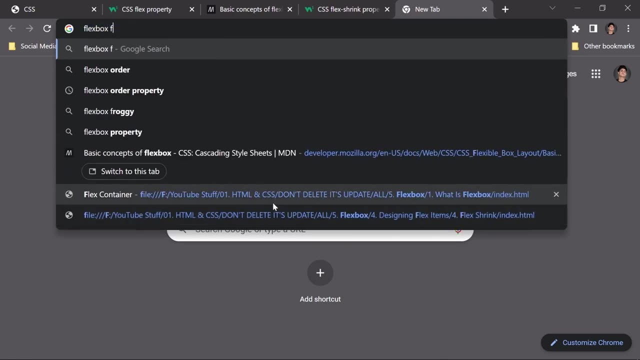 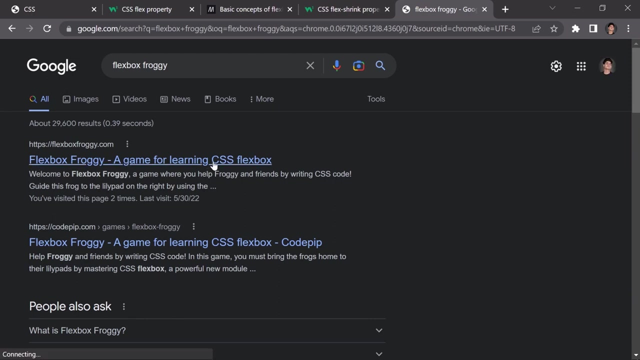 string property. so now it's time to play a cool game by using a flexbox. so we are going to be putting all of our knowledge into this game. so first of all, let's just go to our flexbox. uh, froggy, froggy, like so okay. so now i'm going to just click on this flexbox. froggy again for learning a css flexbox. 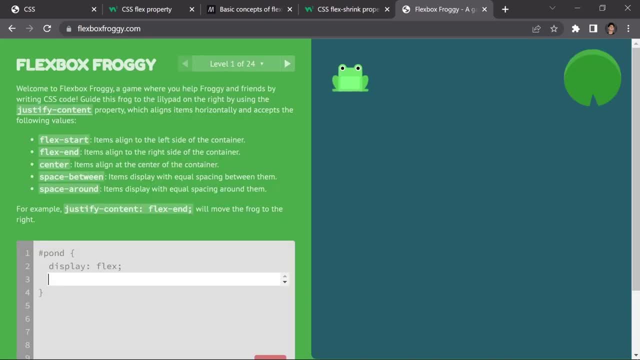 so i'm going to just click on that. and now here, what do you have to do first of all? first of all, you just have to read through this instruction. but i'm going to just click on this instruction, not going to read through this instruction, i just know. i just look at the layout and i'm going to. 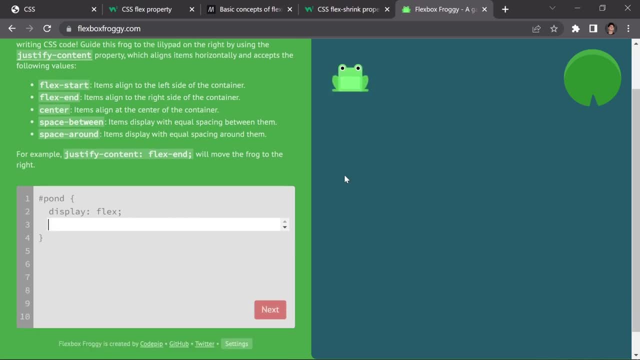 just type a code for that. so i know that. what do we have to do now? our main axis is now set to row. so what do we have to do? we have to just write a justified content of flex n, and if you just do that and push it right there, certain law just allows us to the next level. like to go to the? 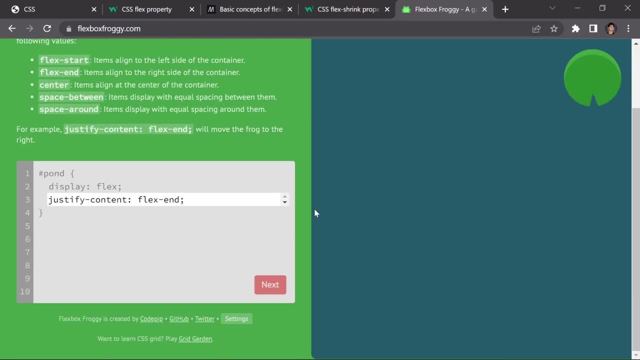 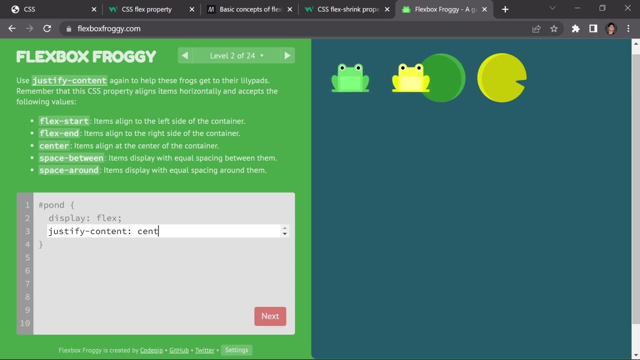 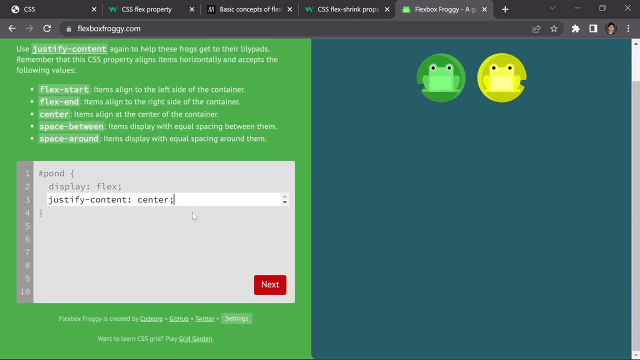 next level. okay, so if you just click on there? so now the next level which we are going to be doing is something called a justified content, content of center. so if you do that, it will now push over frogs to these uh, whatever that has a leaf, whatever you want to call it. now, second mission is also complete, so i'm going to click. 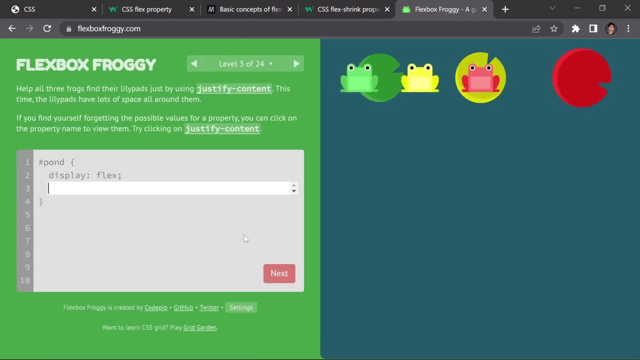 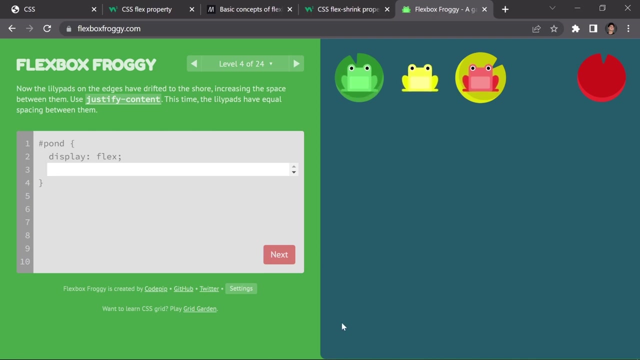 on that. now, what do we have? we have a third one. now let's just try to justify content. it's kind of a simpler. so you're going to be using, like, space around- uh, is it around? yeah, it's around. so we want the spaces around this item and now hit next and boom. now what else do we have? we have to. 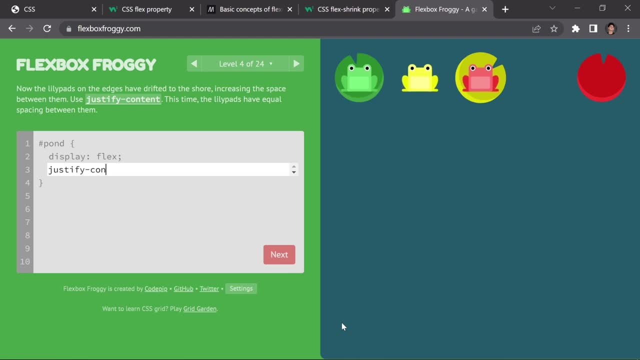 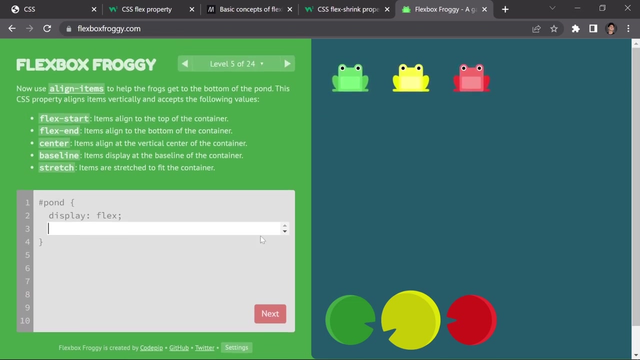 do is we are going to set the content of space between inside there, so justify content of space between. okay, so now this one is also done. we are now at the fifth level. so now it's uh requiring us to work with just uh alignments. we are going to be using, like uh, flex direction is there, so align. 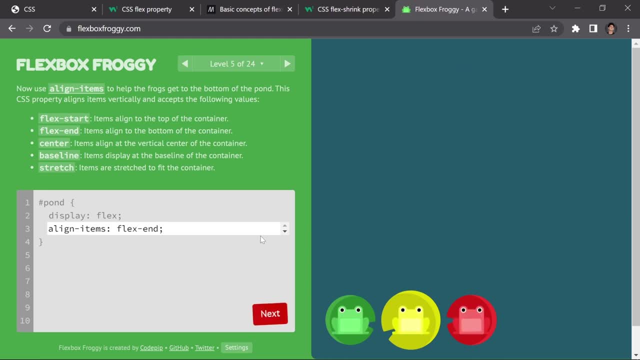 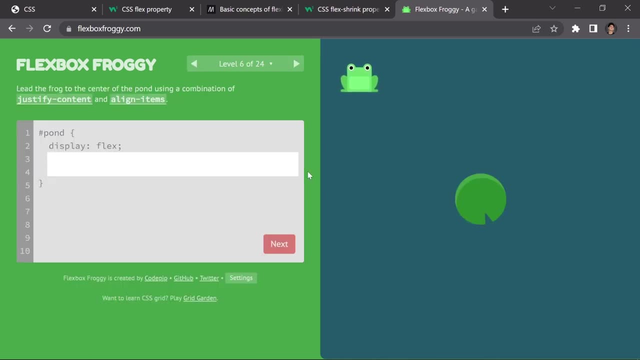 items will be just um, you know what? flex, and so if you save that and boom, everything is working. so now the next. oh, my goodness, it's like the hardest one, it's not? we already learned that. we already learned that- how to do this layout- during the coding tutorial sections. we are going to be 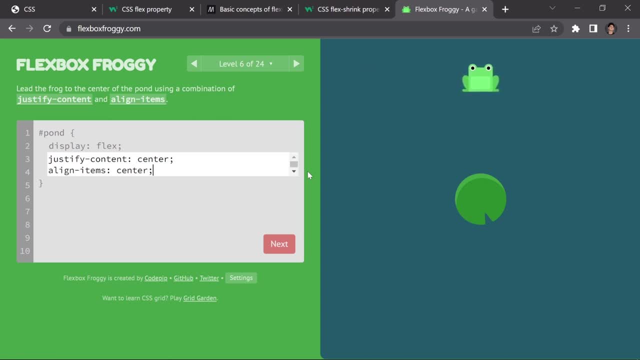 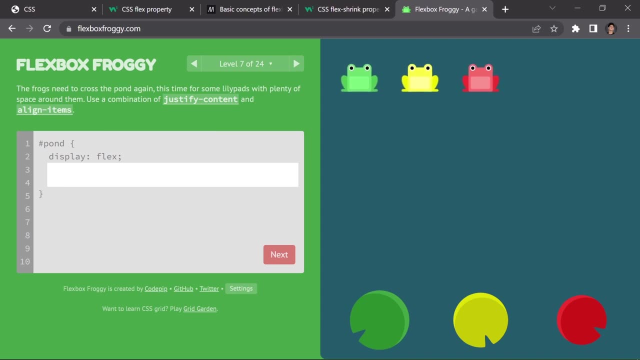 writing. justify content of center. aligned items will be also set to center. okay, so both of them will be centered center. so it will now make us gives us totally perfect center, okay, so now, what do we have? justify, uh, justify- content will be now set to like space, uh, between, i guess. 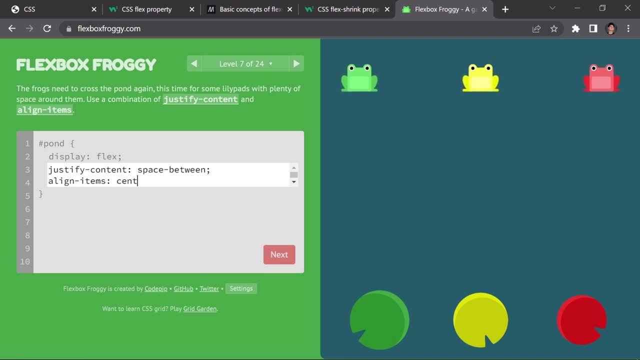 yeah, and then align items will be now set to sin, not cinema flicks, and okay. so now it's okay, it's not a center, uh-huh it also. i guess this one is a center. you know, you just write center. now it's not a center, it's a space around. i guess, yeah, that's a totally space around. now we have to. 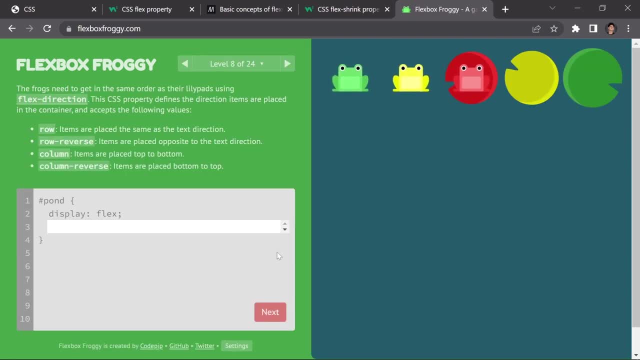 click on the next one, and now this is looking a bit weird. we have to reverse the first one, and then the second one, and then the third one. so what do we have to do? we have to just write like: uh, i don't know, uh-huh, we have to just write, i guess, a justify column: reverse, uh-huh, let's just. 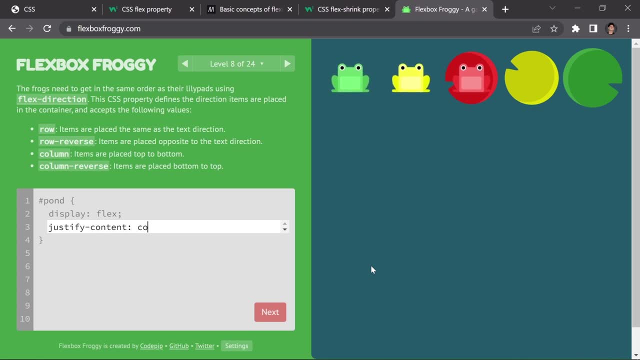 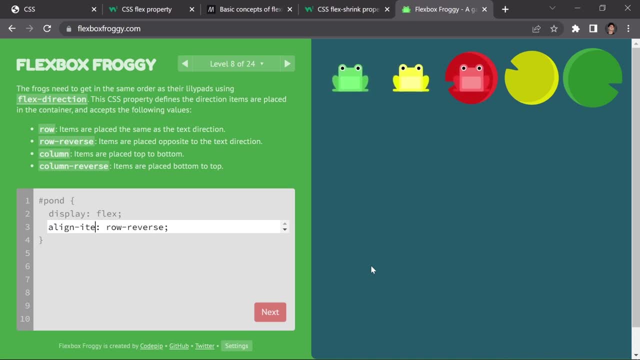 justify content. it should have to be align items. okay, it's not aligned items. come on, man. flex direction of uh, d-i-r-a-c, d-i-r-a-c-t-i-o-n of row, reverse, like that, okay? so, oh, my goodness, i'm gonna just right click on it and make a direction, and now we are totally done. so now let's just hit. 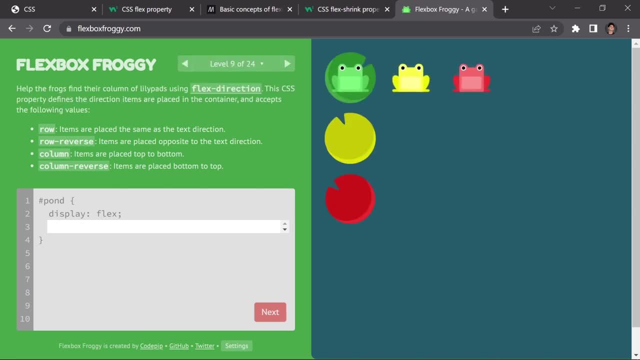 on the next one and i guess i'm gonna have to stop, uh, playing this game, because this is a huge game. okay, now let me just try and type it out, and it should. and this one is easy. we just have to write like: flex, our direction of column d-i-r-a-c-t-i-o-n of. 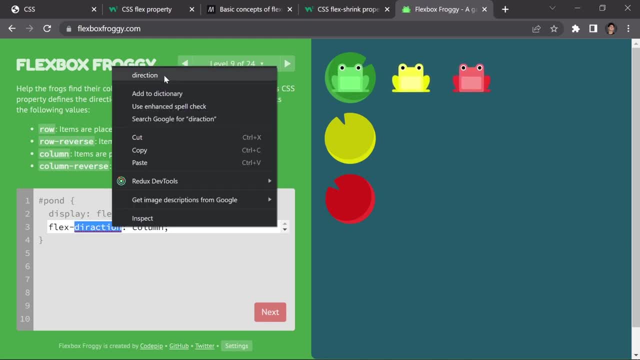 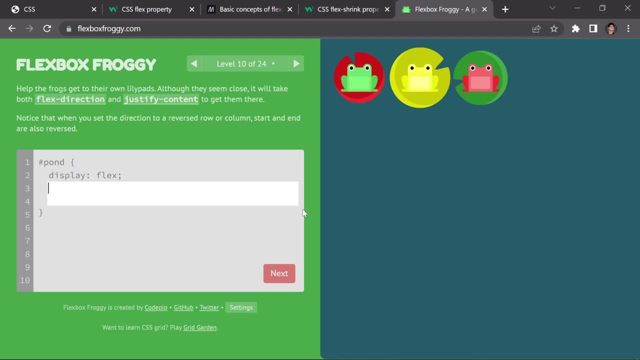 column. why the hell? d-i-r-e-c-t-i-o-n? come on, man. yeah, so that's cool. now the next one we have is, first of all, we have to write a flex direction to row reverse. so i'm going to just write like flex direction to d-i-r-e-c-t-i-o-n, in this case of row reverse. 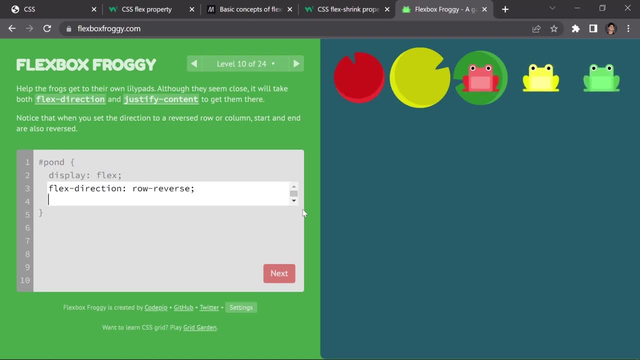 and then yeah, and now we reverse our item. so now we just have to start it from. justify content of next: uh, start, okay, okay, so it's already started. we have to use the end one. yep, that's cool. now hit click on the next one. and now this one is a little bit tricky. 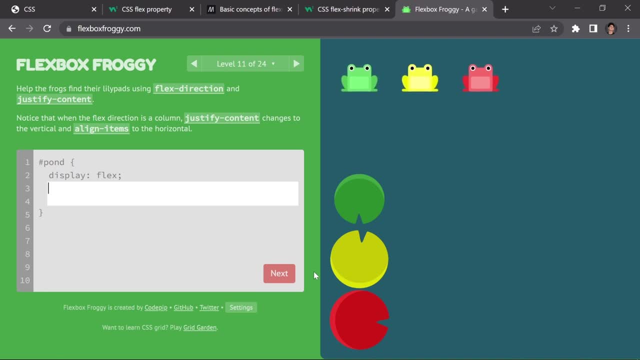 so now let me just have to think about this. how am i going to be solving that? first of all, we would need to write this: uh, flex direction- that's obvious- of column. and now, what else do we have to do? we just have to push that to the end. so justify. 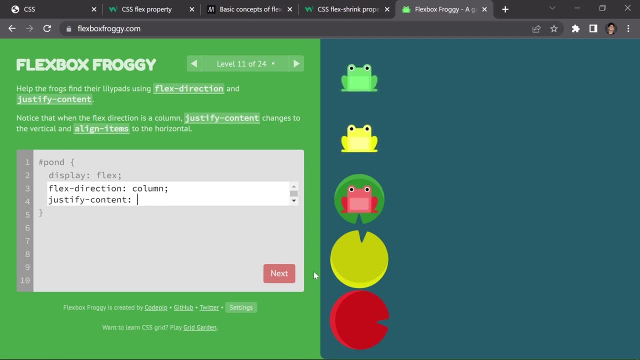 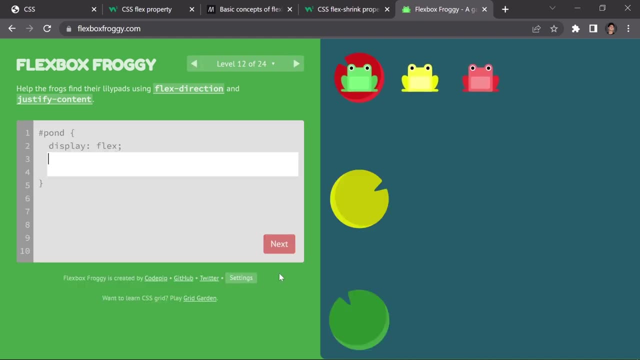 content and there's going to be flex. oh my god, flex n. okay, and boom, we are now at the 12th challenge. okay, let me just think about this one for a second. uh, okay, so how can we solve there? um, first of all, let me just write a flex direction: t-i-r-e-c-t-i-o-n of row reverse in here. 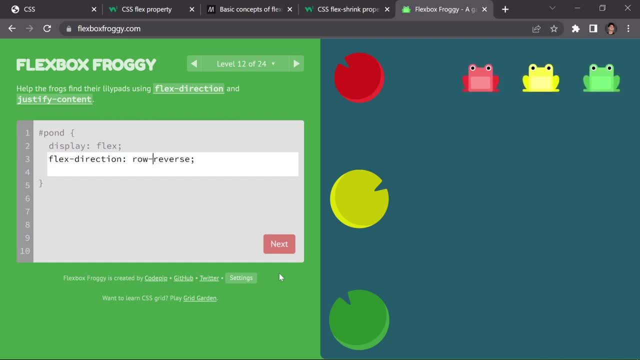 okay, that's bad. ah, instead of row reverse, we can also do like column reverse. that's cool. now the next thing which we have to do is that just write like space between yep, justify content will be just space between and doom. okay. so we are now at the 13th challenge right here and this: 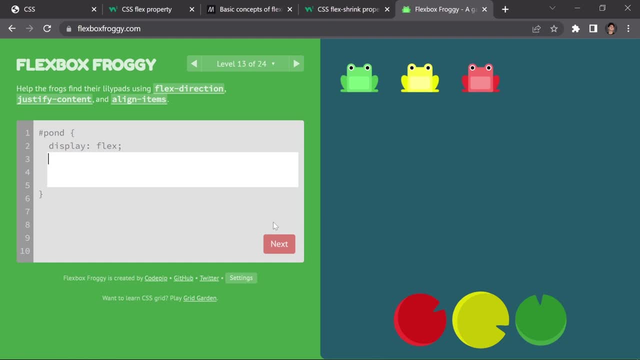 one is quite obvious. this one is totally the easiest one, in my opinion. so what do we have to do? first of all, we just have to write a line: items of center- not center, but flex, and because we want them to be at the end, okay. now the next thing which we have to do is that we have to just write: 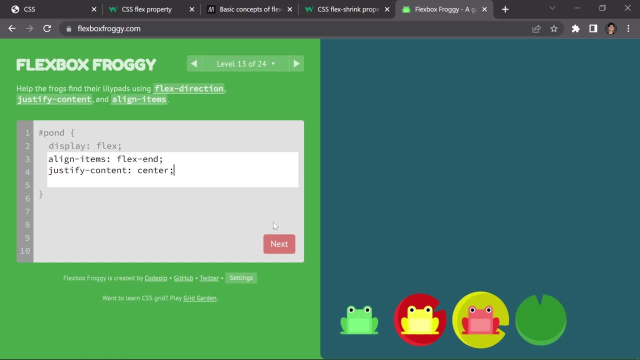 like a justify content of just a center. so you want everything to be perfectly centered? uh right, all right, all right. so now we just have to, uh, change the direction to be like: uh, something else. you know what? i will rewrite this code and it work. so now let me just write like a flex. 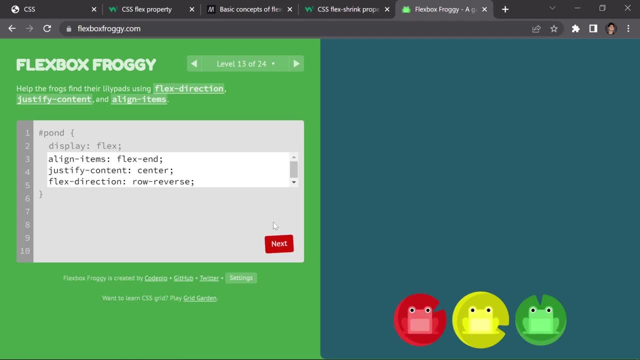 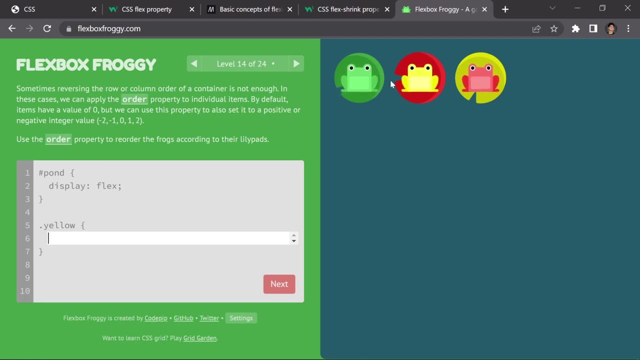 direction of row and then reverse and boom. it will not just reverse it right here. now let me just write: hahaha, we just have, i guess, reverse that, or don't we? okay, so instead of: so this one will have zero one, one have zero one, this one will have zero one. so we have to select that yellow. okay, so we already. 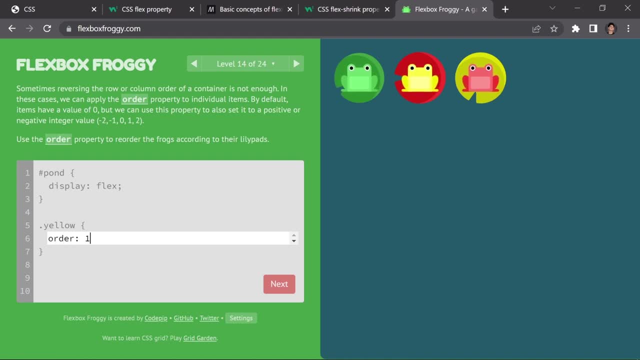 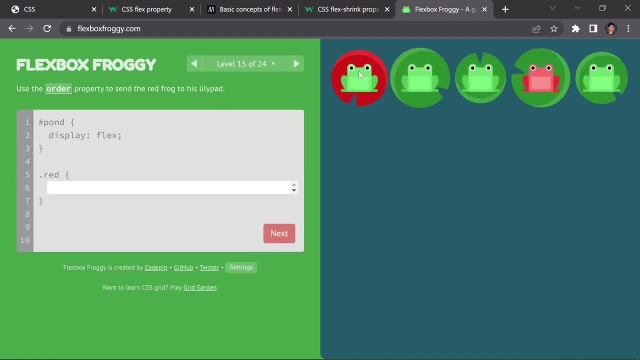 select that yellow one right here, and we are going to be just providing an order of special like one order, and boom, that's cool. and now here, what do we have to do? we just have to. okay, so, how the layout will look like. so we already select this red one and now here, in this case, we are going to be using 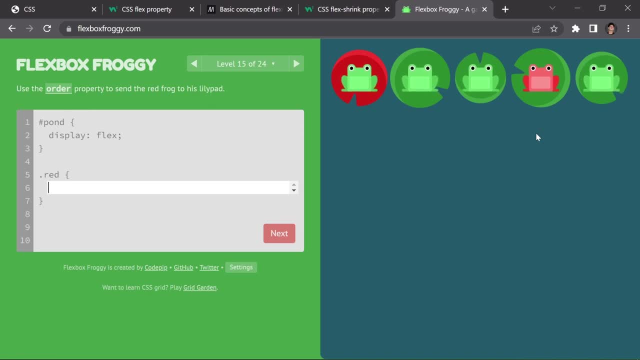 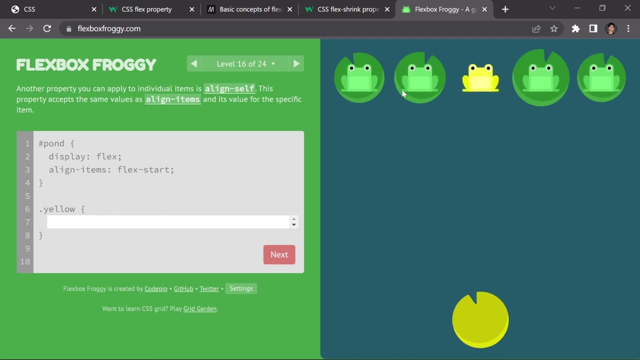 uh, less value than one, so, and even less value than zero, so we can work with that negative value like minus one, like so, and boom, that's got it. that one was quite a little bit difficult for me, all right. so what are we doing in here? these screens are at the green part. well, here we just 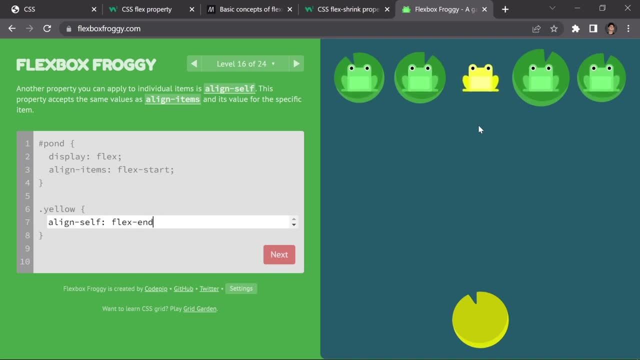 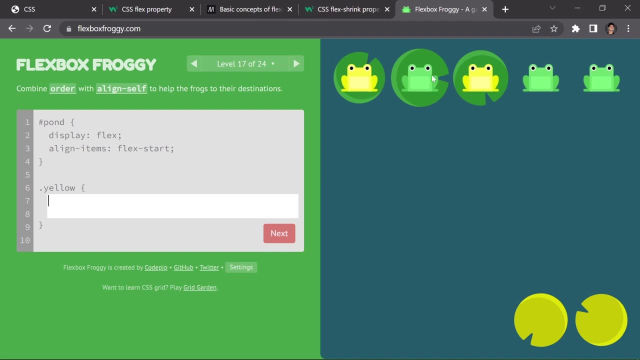 have to use, like align self property, and we are going to be using a flex and and boom, that's it all right. so what are we doing? first of all, we are going to make these two up here and then push it down, so i know that we are going to be using uh. 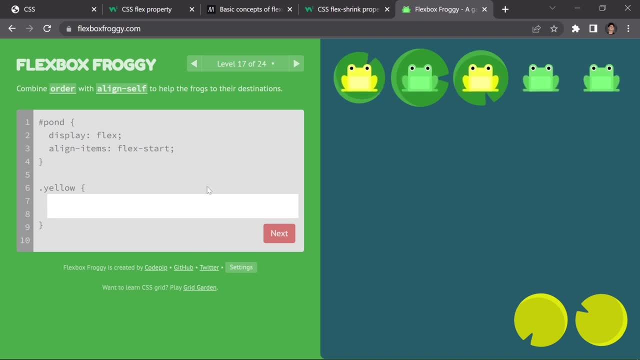 align self property and we are going to be using, uh, align self of n. we already select a yellow, so now let's just use this align self of n. so i'm going to write like: align self of just a flex, and it will not push it right here. now, what else do? 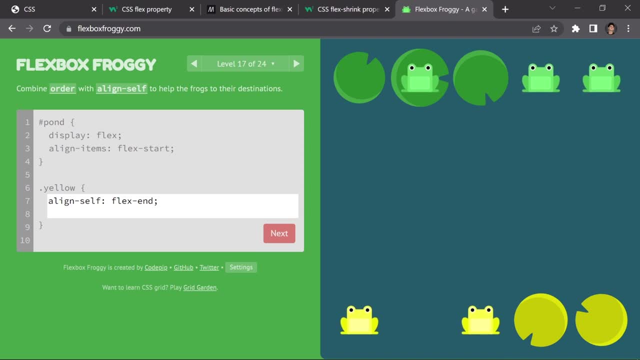 we have to do? do we have to just write: uh, justify content or flex? start will be n. let me just think about that for a second. i don't know how we would solve that. this one is like the most trickiest one. okay, yep, we can use the order one, so let me just write order. property of one. 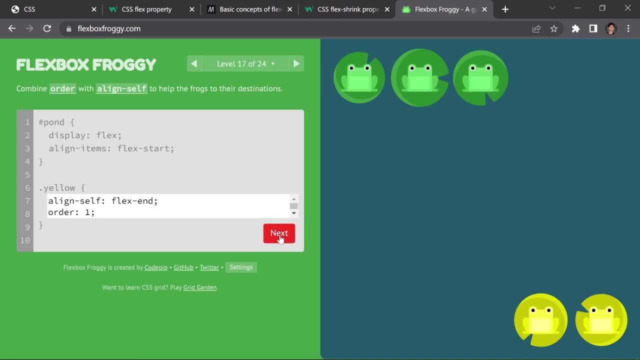 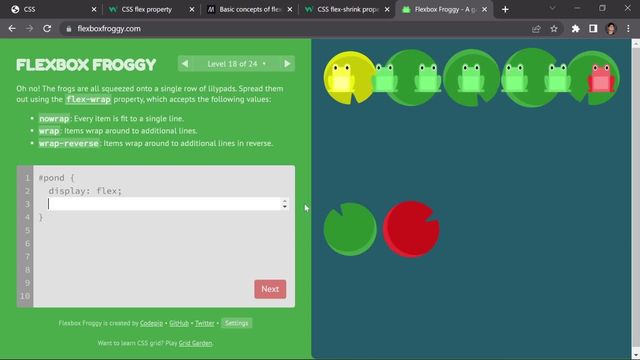 and boom. okay, so now everything is at this end and that's it all right. so this was kinda a little bit uh getting all right. so these challenges are getting harder and harder. so we are now at tn, so we have to figure out how to solve that. so okay, so they are squashed together to each other, so let 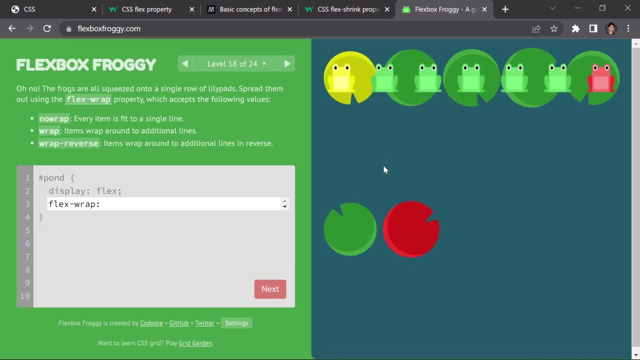 me. just try to wrap, that let's wrap. and by default value is no wrap. so i'm going to just write like wrap in here, and then i'm going to just write like wrap in here, and then i'm going to just write like wrap in here. 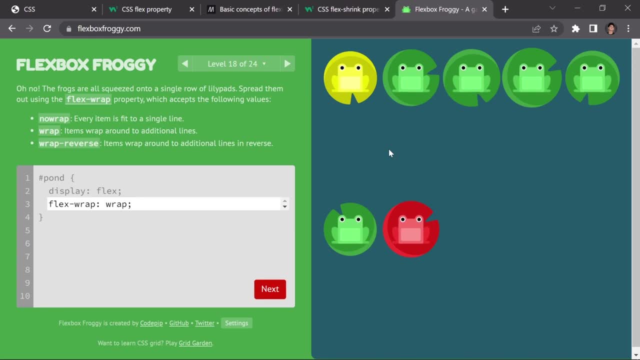 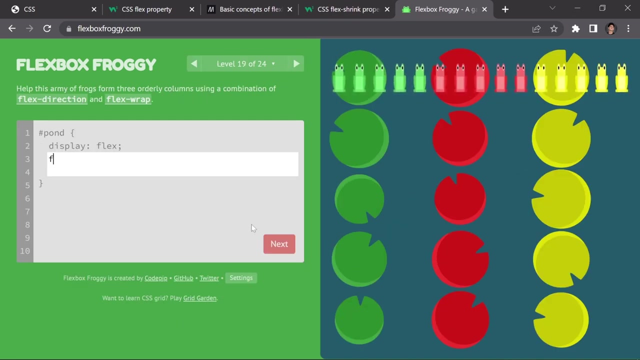 here and, yep, i get, that was that one was quite simple and easy. oh my god, all right, so now let's just hit next one. okay, so i know that we have to write a flex wrap first of all, so we are going to be using like a flex, uh wrap of wrap. okay, so we are totally there. 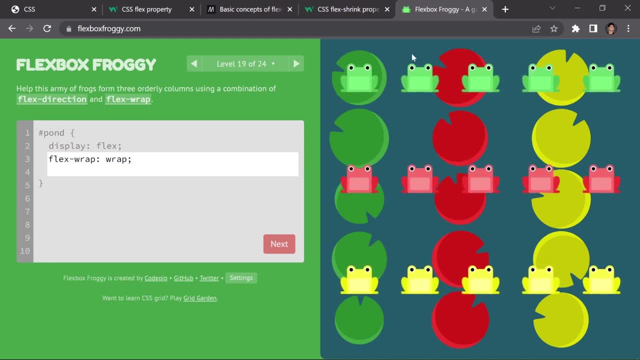 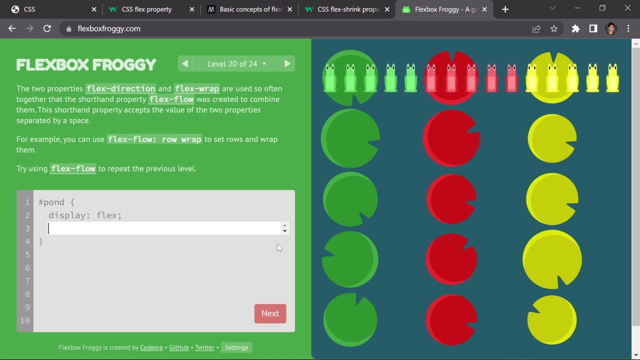 but what else we have to do is that we have to change the rows to the colon- yep, that's cool. you can use a flex direction b-i-r-e-c-t-i-o-n to the column. boom, yep, that's cool. now hit next. and now we are at 20, so i guess, what do we have to do? okay, so, for example, you can use a flex for 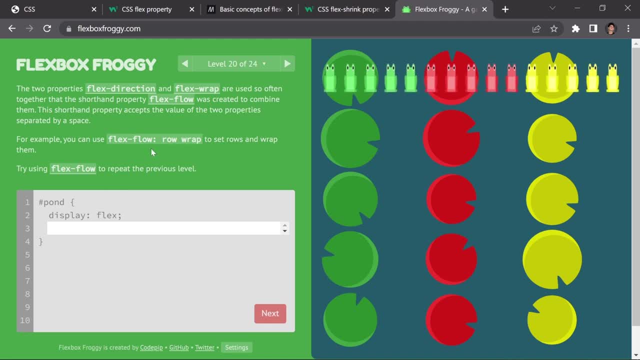 oh, my goodness, a flex flow is just a shorthand for writing a flex direction and also the wrap property. so we are going to be just using like a column wrap in this case, because we want to. you know, we want to use a column wrap in this case because we want to use a column wrap in this. 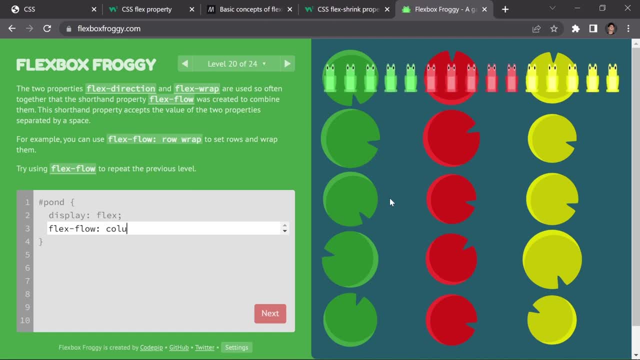 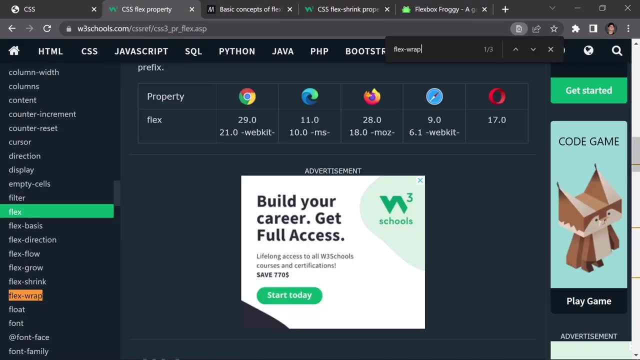 because we want to use a column wrap in this case, because we want to use a column wrap in this case, write that as a column wrap. so flex flow and column and then wrap. so i'm going to, first of all, you show you the documentation of flex flow so that you guys can see everything a bit better. 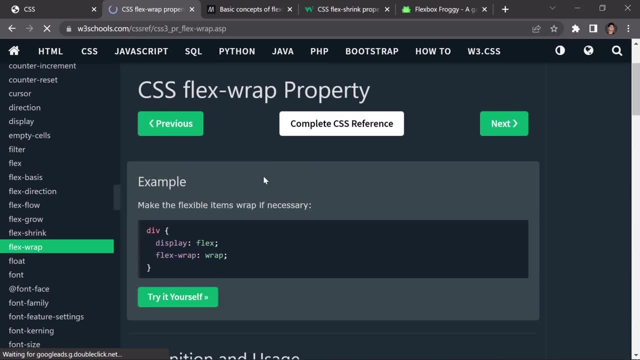 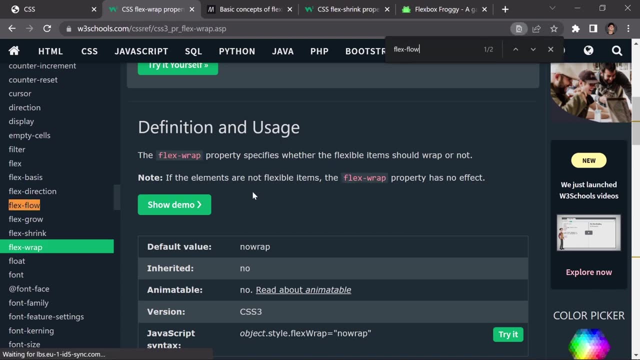 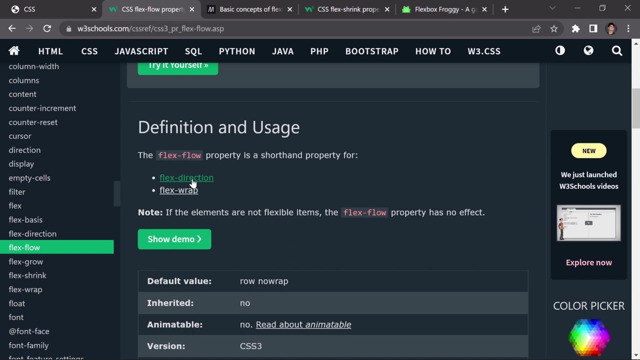 i forgot to show you this one. i was just thinking like i missed something. okay, so the flex- oh my goodness, not a wrap, flex, uh, flow. and this one i want to click on there. and now, here you can see, the flex flow property is a shorthand for a properties of flex direction, which allows us 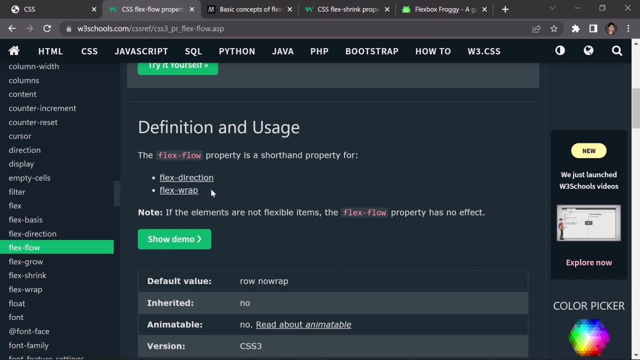 to change direction. then we have a flex ram and it allows us to just either wrap or no wrap or wrap rewards items. so there is just a shorthand for using a flex direction and flex wrap. i apologize about that. i didn't show you that in the first place, but now we are at 21 project. uh, i. 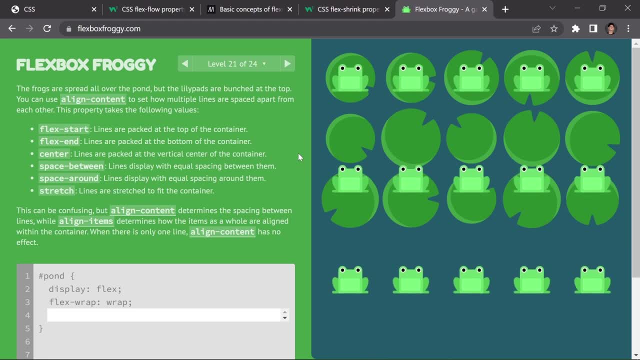 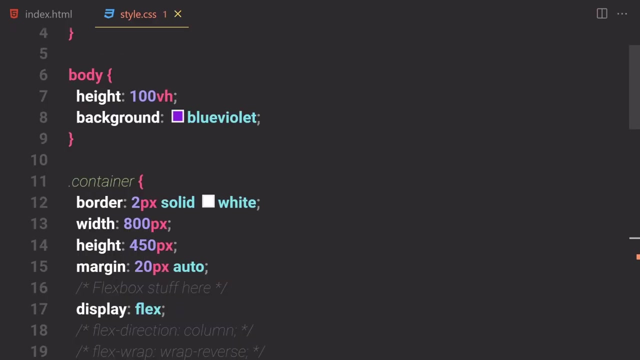 mean like 21 challenge. so what do we have to do? first of all, let's just read through this instruction. uh, okay, so what do we have to do? we just have to remove these empty spaces from there and yeah, but there we are going to be. i guess using align content property. did i show you a line? yeah, 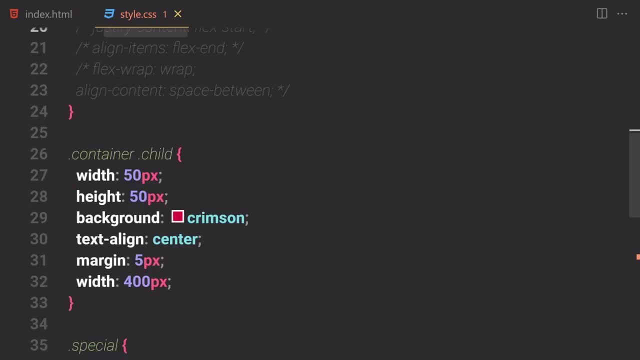 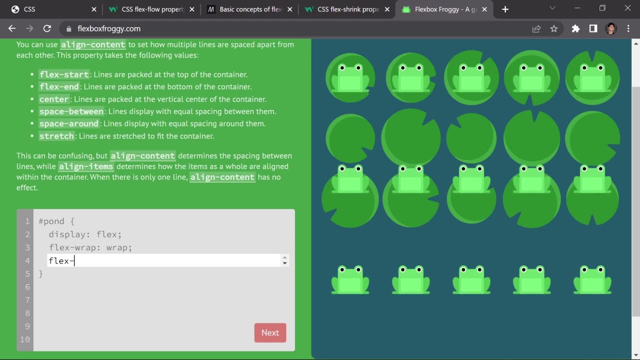 i did show you a line content problem, not this one. where is a line content? yep, right here, space between. so here we are going to be using flex, uh-huh, not flex. so here we are going to be using just a line content. property of flex start. okay, so let me just write it like: flex start and boom. 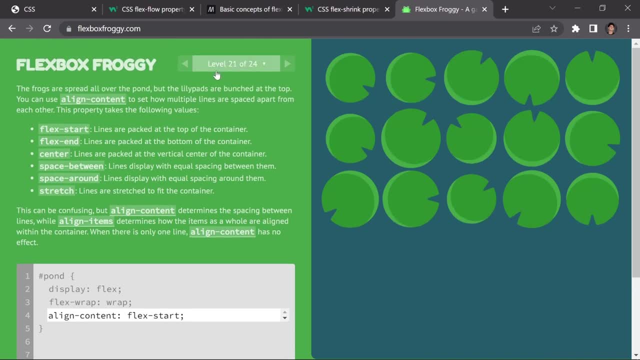 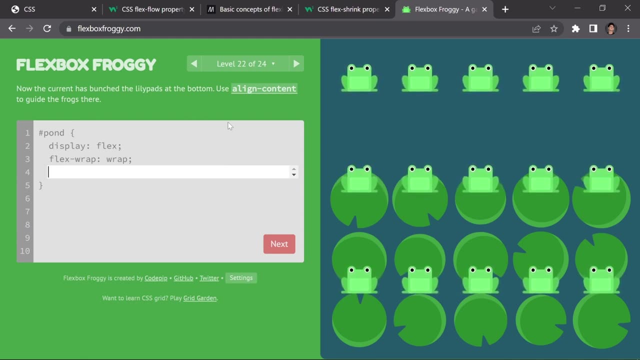 okay, that was also a little bit simple. so we are at 22 and now let's just figure out, like, what do we have to do in there? okay? so this one is a little bit. okay. so we have a lot of content we want to push test. so we can use align content property, as they said, so we can use. 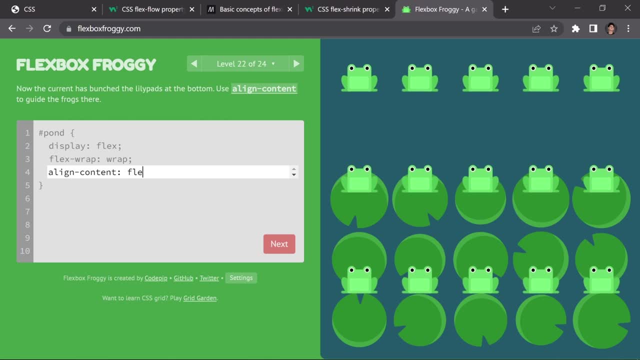 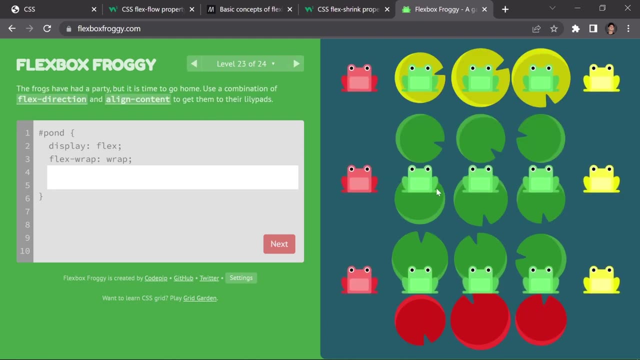 align content property and we can use like flax and and boom. everything is working. the way we experiment work. and now this one is a little bit tricky, to be honest. i'm gonna have to to just wait for there and just check out this layout. okay, this one is a little bit tricky one. 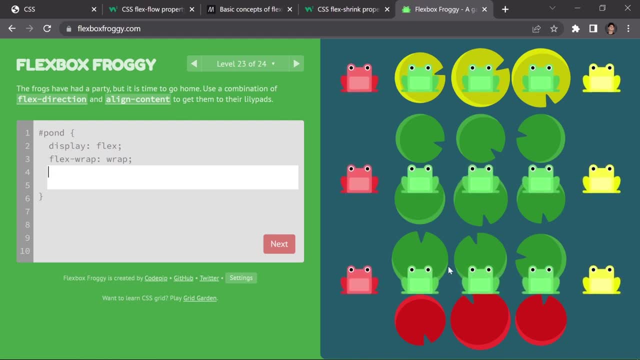 so what do we have to do? we have yellows in here, then we have a greens in here, and then we have red. so you know what? uh, okay, so display will be flex and flex wrap will be set to also wrap, so it's now wrapping itself. so now, what do we have to do? i know that we have to change the direction. 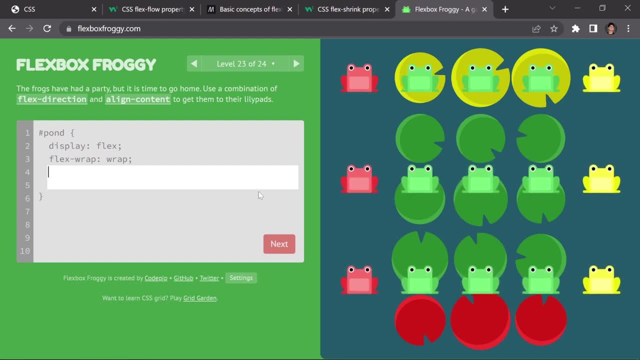 and we can do: uh-huh, we can do a row reverse. yeah, we can do a row reverse. so flex direction will be set to like d-i-r-e-c-t-i-o-n of row reverse. okay, all right. okay, that's awful. instead of row reverse, let me just write a column reverse. yeah, we are getting there and now we just 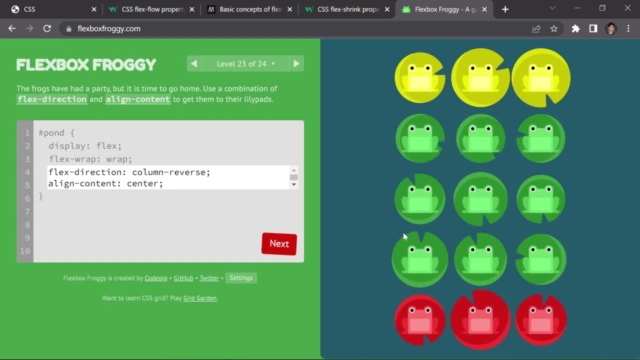 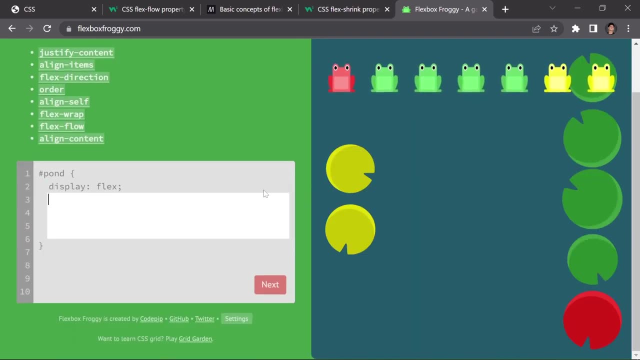 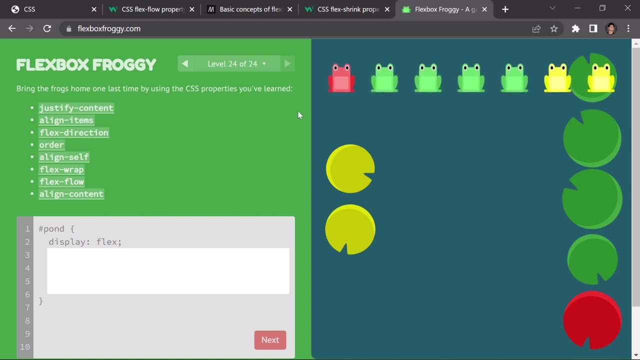 have to use align content of center and boom, that's cool, okay, okay, uh-huh, uh. and then we have a final project, okay, okay, so we have to use all of that. okay, so this is the final test which we are going to be doing. okay, so we have first of all the red, which needs to be in here. i guess we can use a flex. 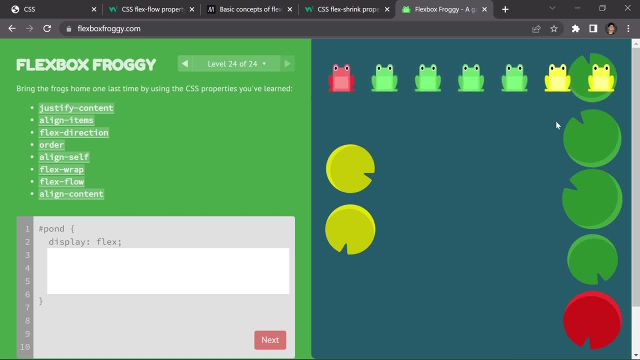 or align cell for that. and then we have a greens, which needs to be in here. then we have two blues or not blues. we have two yellows, which needs to be in here. okay, so they just provide a display of flex. come on, we have to figure it out. what do we have to do? uh-huh, first of all, let's just start. 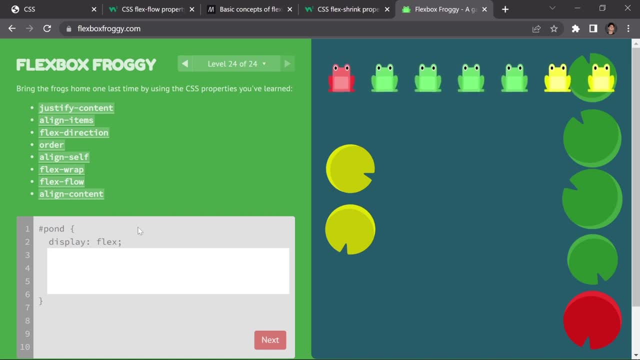 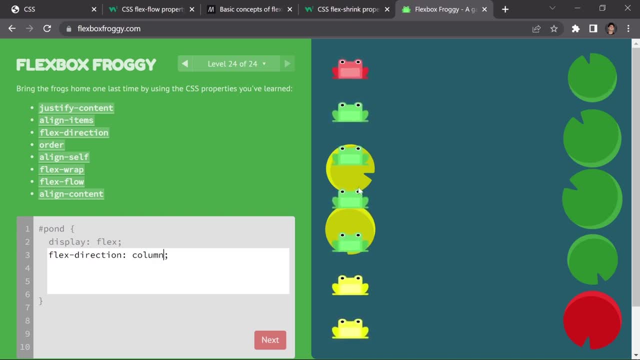 mn. so this is now colon, so we can now push this item to in here and push this last one. so now, in this case- you know what i'm going to write- a column reverse in this case. so, yeah, we are getting there. so now we can push this item and we have to also wrap that. so if you wrap that, so this item. 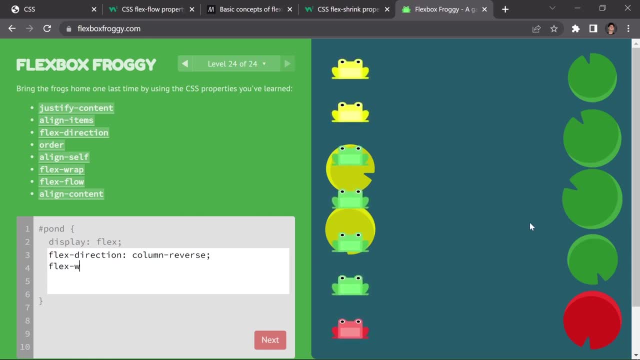 will take its place and so on. so let me just write like a flex wrap of just simply a wrap. okay, um, i guess we have. we want this item to be in here and the other item to be inside there, so we can write a row: uh, wrapped reverse for that. so wrap reverse. and yeah, that's looking cool. but 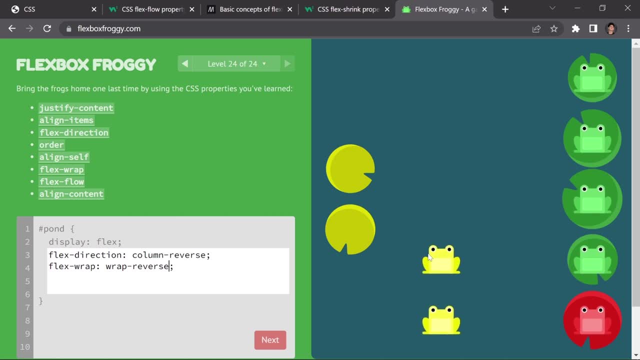 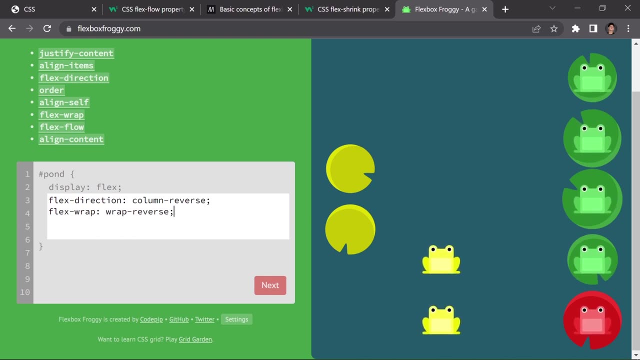 what do you have to do for this ones? okay, so i'm gonna which kind of center properties we have. we have a line center and we have justify centered, so justify content center. um, what, what in the world can i do right now? so you know, i'm gonna just write like, first of all, just 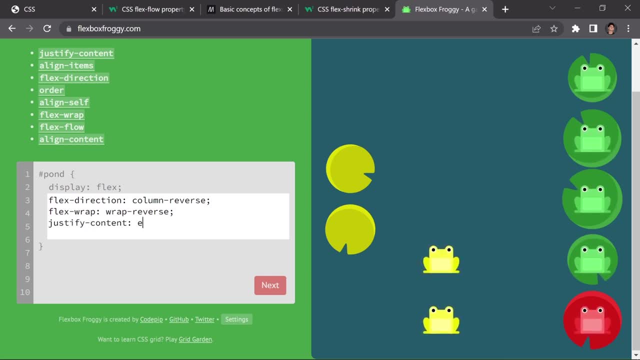 to start with the justify of content of center, because we know we have to center this stuff and, yeah, we are getting there. final property we have to write is align items of center. okay, center and boom, not boom. but we have to just wait, for you know, i'm gonna provide a flex, uh. 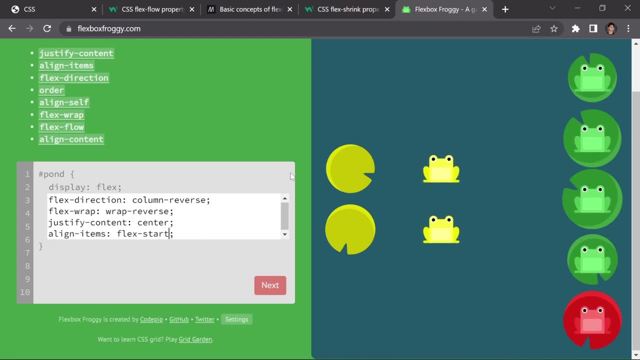 start, start property. this one is a little bit difficult. come on, how can i do that? okay, so we, we can just try like space around property, can't we? let me just start um between. come on, flex between, what the hell? flex between, not flex between, but space, uh, around property. 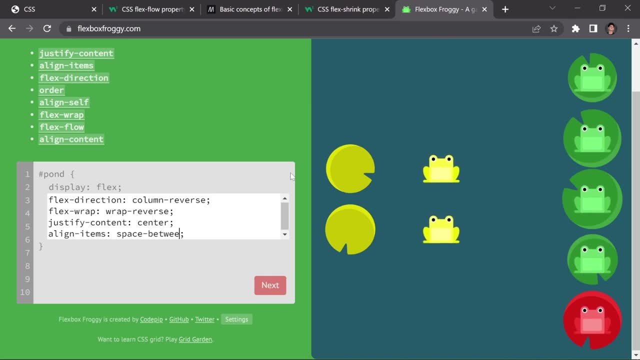 okay, it's not working. let me try a bit. we are not. yeah, space between come on align items is not working. okay, so we have more than one item, so for that we can use, instead of align items, we can use align content right here, so we can. 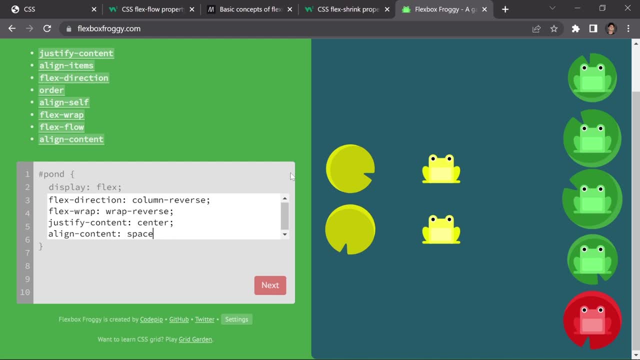 just write like space, uh, oh my goodness, space around in this case. and yeah, come on, oh my god, so, okay. so now we are getting there. so instead of using around, we can use between and boom, come on, we are now totally done with this challenge and we did all of them, so level from 0. 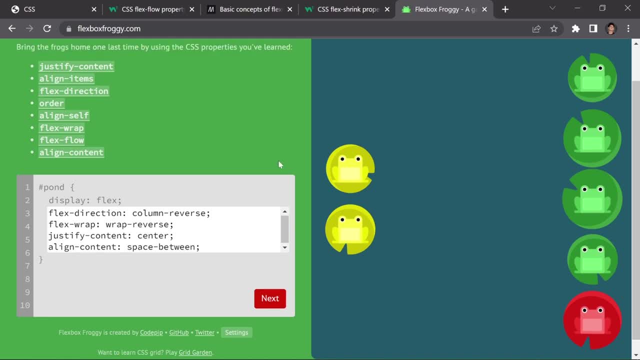 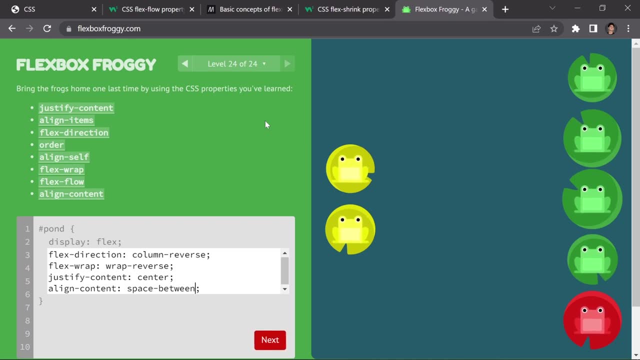 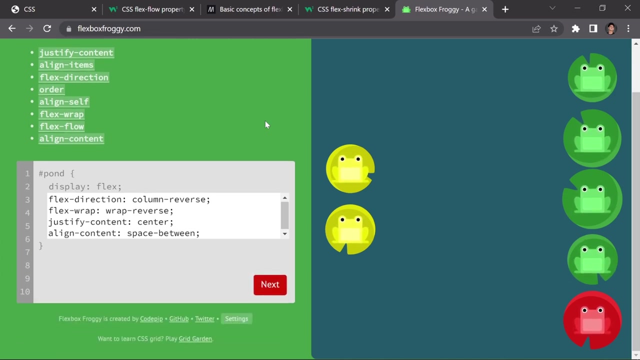 through 24- 24 to be precise, not 25- and congratulations. we learned about flexbox and now you totally master flexbox. now the next thing which we have to learn is a new css more, which is known as a grid, uh, display of grid, so that one is a little bit tricky to learn. 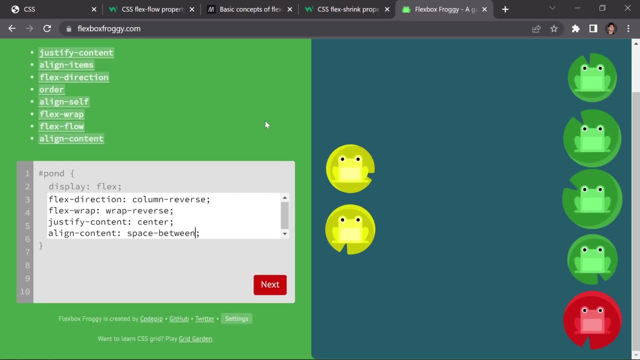 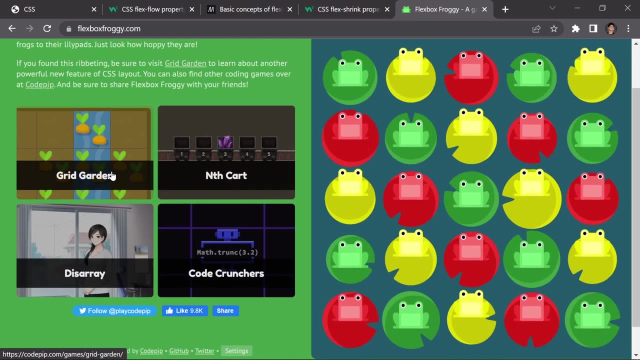 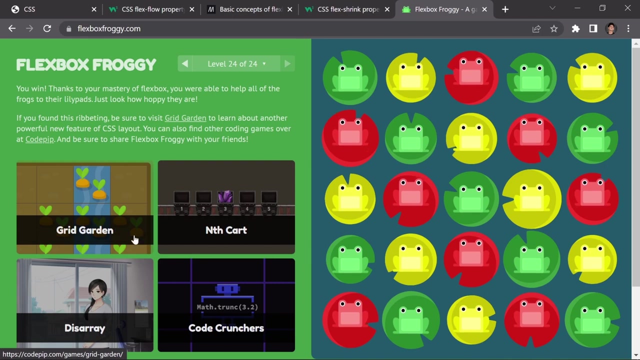 but you have to be a little bit patient and you have to practice that by yourself. and thank you for watching, and i'll just you in one more second. okay, so this is a grid garden. then we have a net card and then a few more- uh, coding kind of challenges. so next we are going. 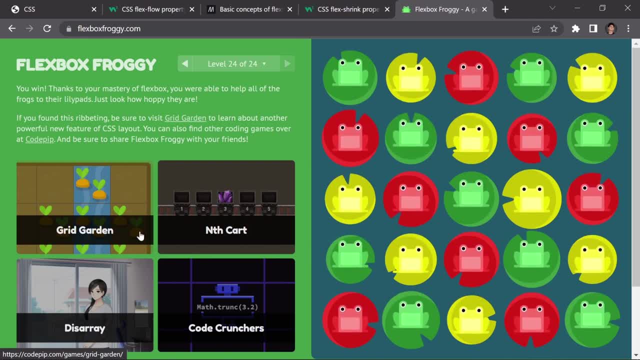 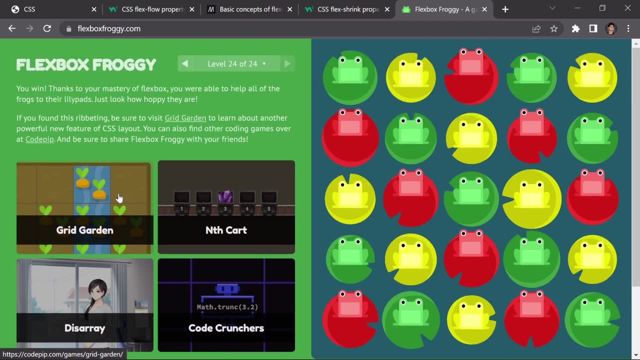 to be working on, i guess, a grid garden, but i'm not going to be playing around with all of the levels, because the flexbox is a little bit easy, but grid is not that much easy. i'm not saying that i cannot solve all of them, but it will take me a lot of time to solve them. 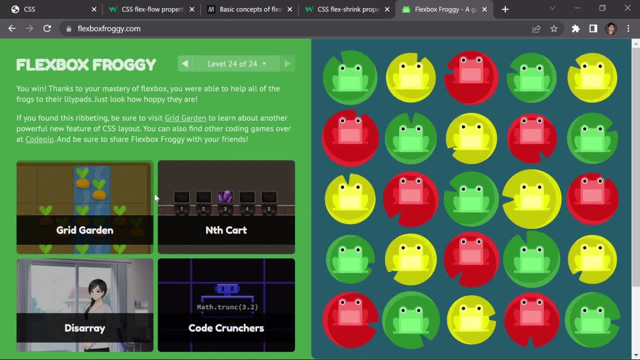 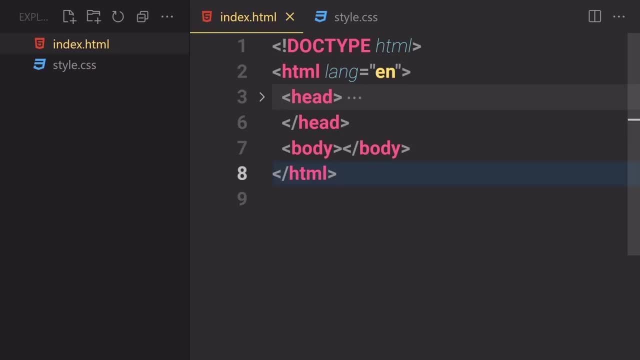 and i don't want that. just want you to learn stuff. i don't want to waste your time and mine as well. all right, guys. so now that we are totally done with the css flexbox layout model, now the next model which you are going to be learning in this video is something called a css. 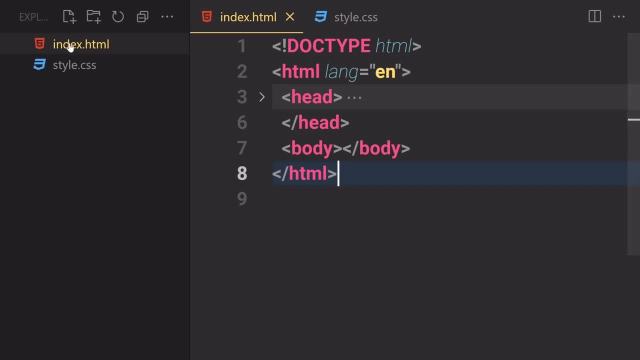 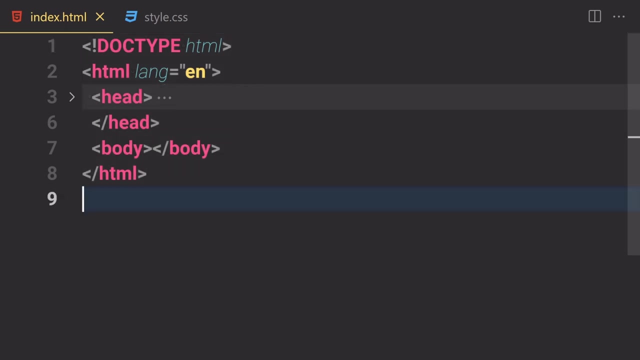 grid layout model. and so here you can see, we just have our indexhtml file and we have just our basic structure of html right here, and then we have our stylecss file and no content, nothing. here you can see, our body is not totally empty. so before getting into the coding, first of all let me 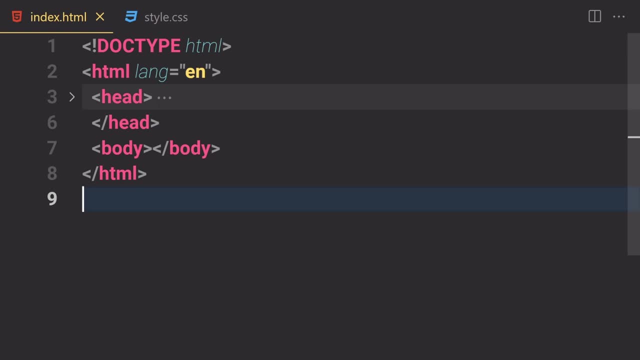 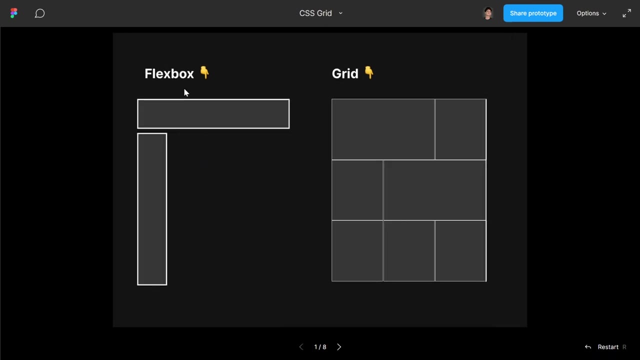 just show you a few slides and then you'll get to know what a css grid is. okay, so then we are going to be writing or coding. we just have to start from the first thing, which is known as a css flexbox and css grid. so a css flexbox, as we know that it will, allows us to only work. 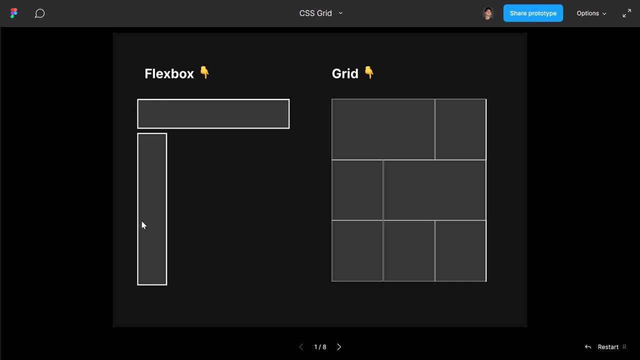 on a one dimensional like, it will only work on a row or on a column, okay, so it cannot work on a two-dimensional layout. on the other hand, now we are going to be learning about something called css grid, and css grid will allows us to work on a two-dimensional layout like. we can set how many. 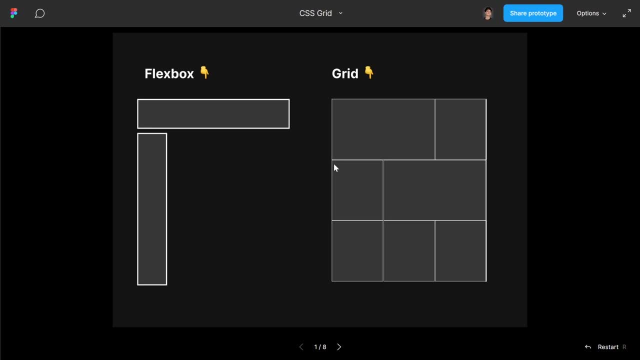 rows and how many columns we want, and stuff like that. so for now, i want you to just remember that css flexbox allows us to work on only one dimensional layout and css grid will allows us to work on a two-dimensional layout. okay, so before getting into the coding, first of all you 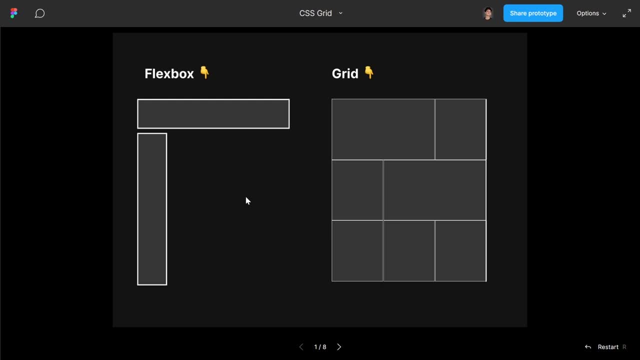 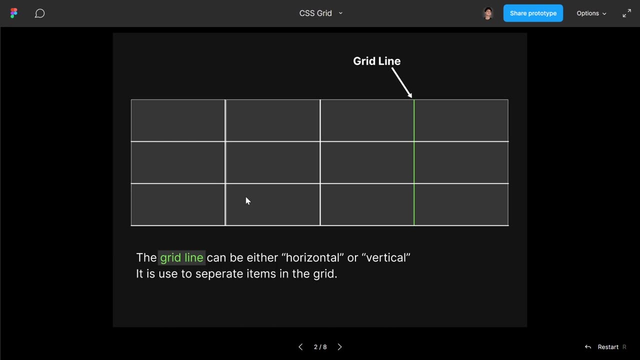 have to understand a few things about grid, and then we are going to be jumping into our visual story code and we are going to be writing a lot of code, all right, so what is a grid line? first of all, so a grid line can be either horizontal or vertical. it is used to separate items on the grid. 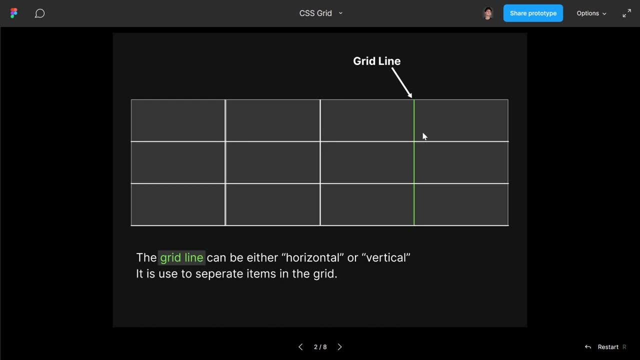 so this one is a grid line, this one is a grid line and this one is also a grid line. these are known as a grid column line and these are known as a grid rose line. right here, okay, so you just have to remember that for now, like you just have to remember this line, like what? 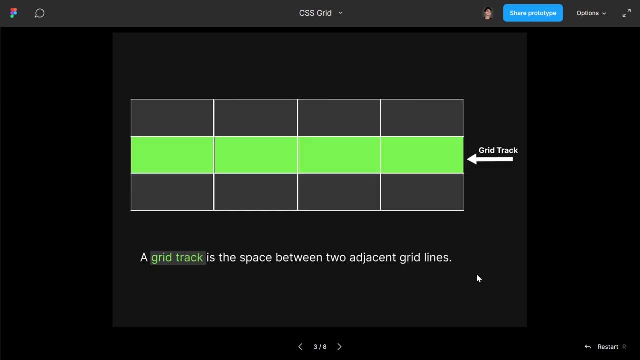 is the css grid lines anyway. so now let's just learn about something called a track. what is a track? so a grid track is a space between two adjacent grid lines. you just have to remember there, and i've highlighted that on a green color right here. okay, so now let's learn about something. 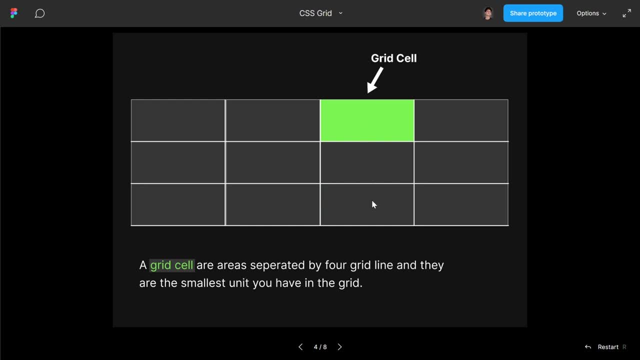 called a grid cell, and we already know that. if you have ever worked with a um, what do we call it? msxl? so if you previously work on msxl, so you definitely know that for sure. but if you don't, so grid cells are area separated by a four grid lines and they are the smallest unit you have in. 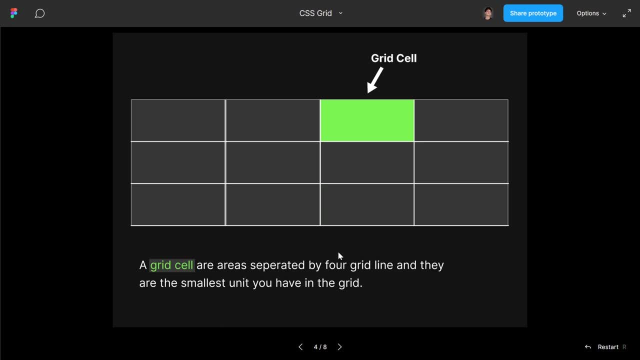 your grid. okay, so you just have to remember that. and now the next topic and the final topic which you are going to be learning in this slide are something called a grid area, and a grid area is one or more grid cells that makes up a rectangular area on the grid. so this is just actual definition. 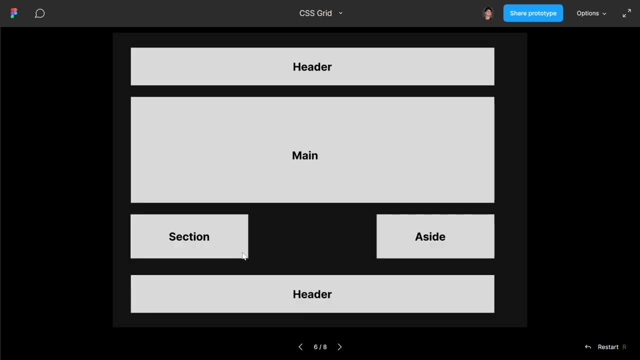 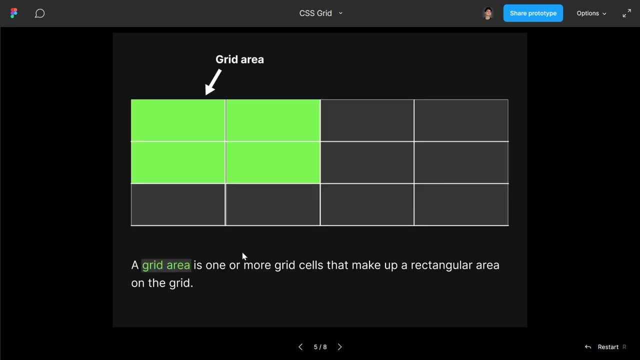 of a grid area and we are out of our slides? no, we are not. these are a few layouts which you are going to be building throughout this section of a grid. okay, you don't have to worry about them for now, but these are a few topics which i want you to keep in mind. 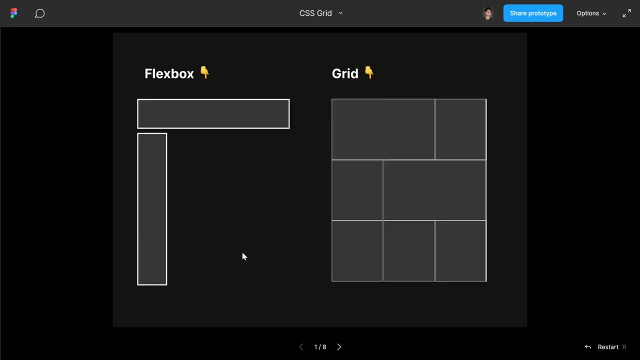 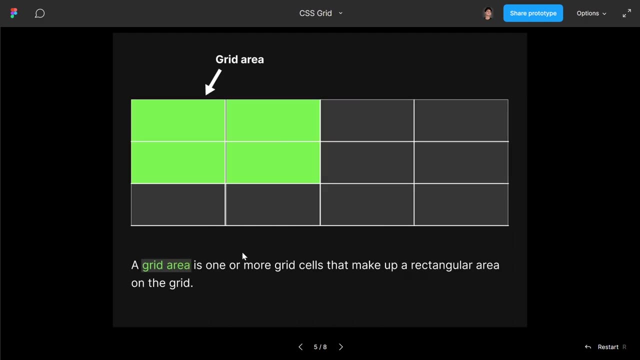 throughout this video. so first of all, we learn about what is the difference between css flexbox and grid, then we learn about a grid line, then we learn about a grid track, then we learn about a grid cell and finally, we learn about a grid area. so i want you to just keep that in mind. 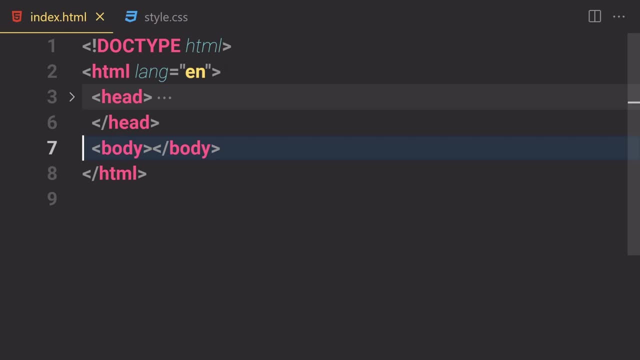 throughout this section. all right, so before getting into the css, first of all we have to write some content for that. so if you want to write our content, so first of all we are going to be just writing a section with the class of container, okay, so first of all we are going to 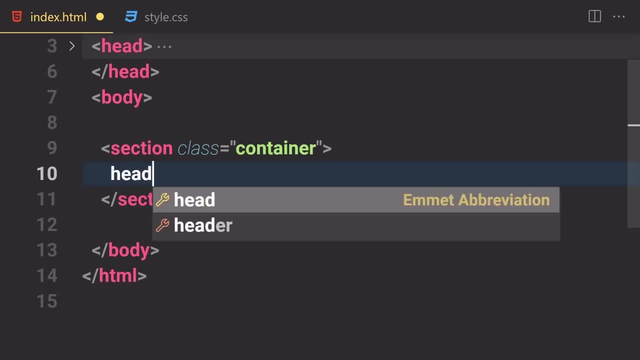 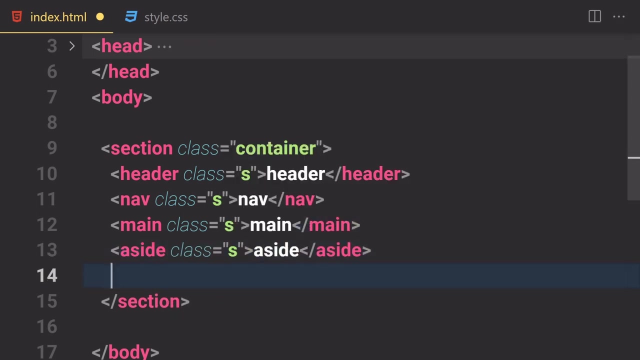 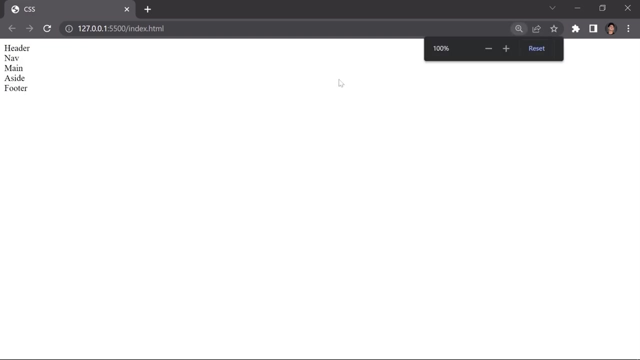 get our css combination right, so CsT, gearbox footer. okay, so now let me just make that a capitalized one, so we have our main, then we have our navigation and then we have our header. so now, if you save that and let me just go to my browser and this is how everything looks like for now. okay, so i'm going to set my browser to 100. 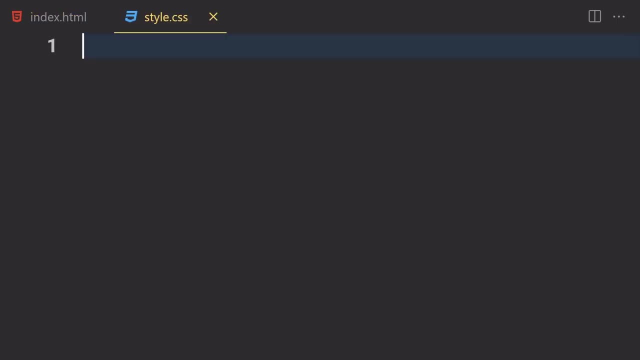 and now let's jump into our css and now let's just write our styling. first of all we have to write our research. like margin will be totally not max resolution, but just margin will be set to zero. and now let's just select our container. and here we are going to be, just first of all writing a 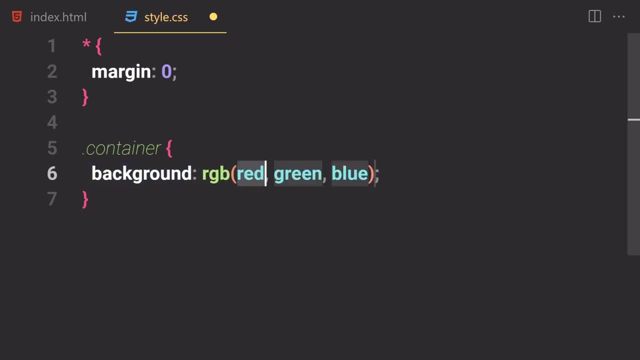 background color of. let me just remove that hexadecimal and set that to rgb and let's just write or 34, 34 and 34 as the colors. now let's just write a padding of 20 pixel in there and i'm going to also provide a height of 100 vh for that. if you save that and here you can see, it'll now take up. 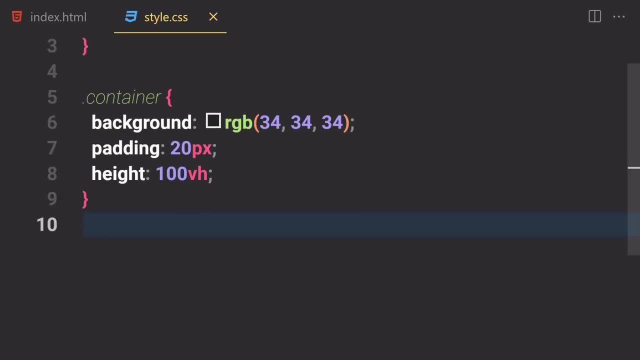 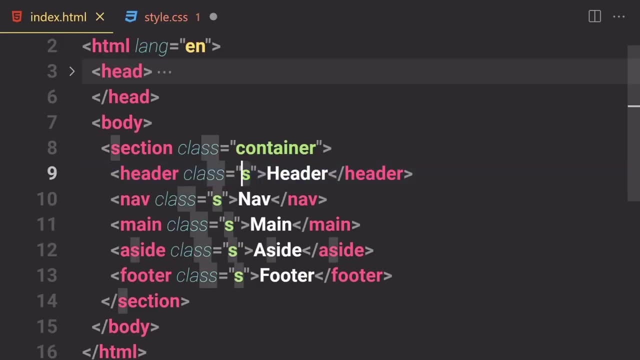 all of the entire viewport height and we will just get a little bit of padding and stuff. now let's just select our s, which is stand for like s which is stand for like a little bit styling, so we just provide this s class to all of these element, or all of these. 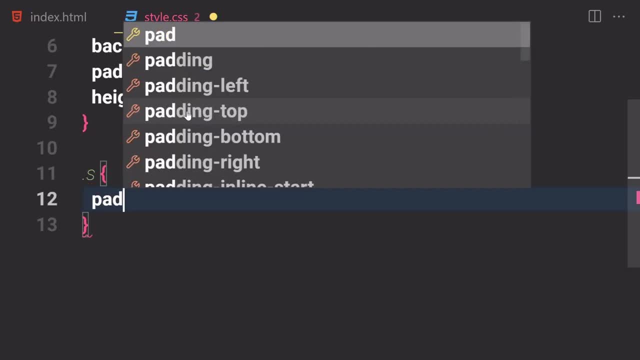 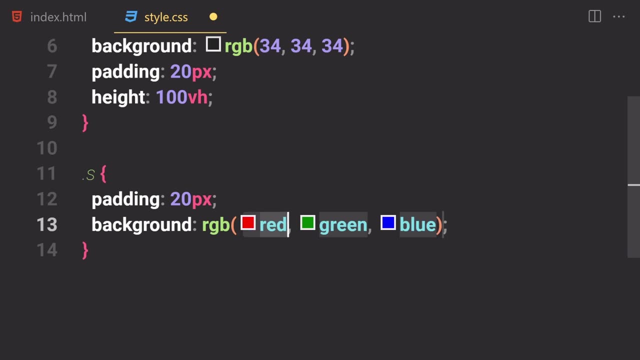 children of that container. okay, so now we selected that let's just provide a padding of 20 pixel in there. background color will be um, i'm going to just provide rgb of 84, 84 and 84. okay, so now let's just set everything like: text line will be set to totally center and text color will be totally. 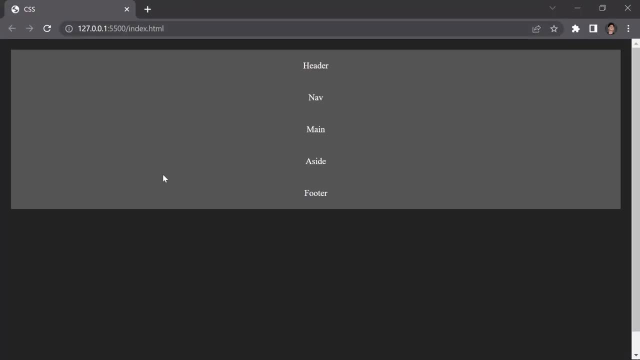 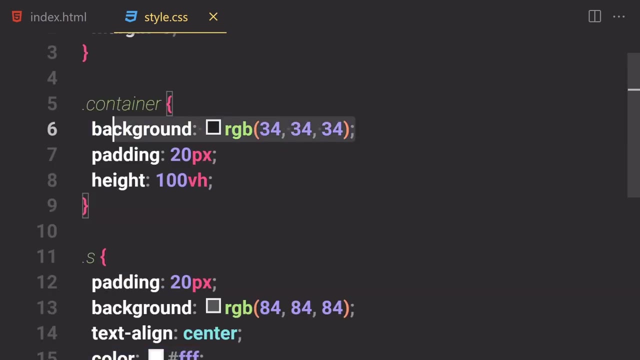 white and if you save that and by default, currently things looks like this: okay, so so here you can see. now you might be asking like, where is our totally, or not totally, but we have like this color right here, so where is that color? that color is hidden inside this s class, so if you 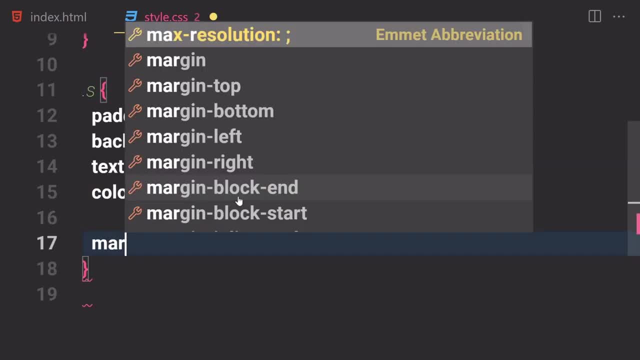 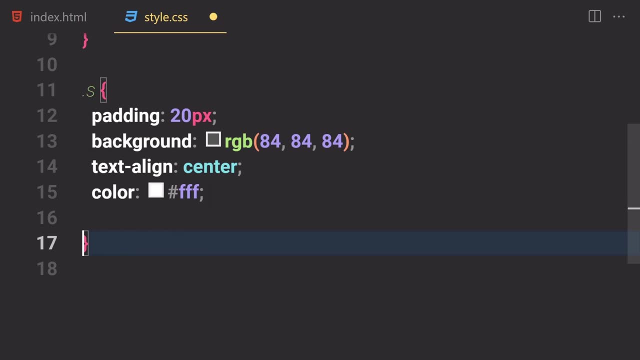 just write. you know, i'm going to just provide a little bit of margin so that you can see that color. i'm going to provide margin of 10 pixel maybe, and if you save that and now here, you can see that color which is hidden on this element. so i'm going to just remove that margin from here. 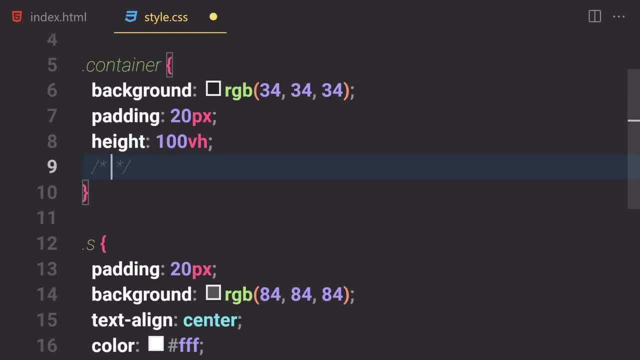 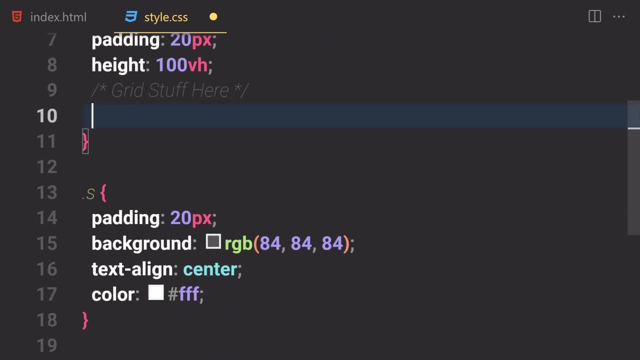 and now let's just start working on our first property. so before getting into that, i'm going to just write like grid stuff here. okay, here come on. so now, as we know that if you want to work with some sort of a display property- like we already learned about a css flex box, so we have to provide a display flex. 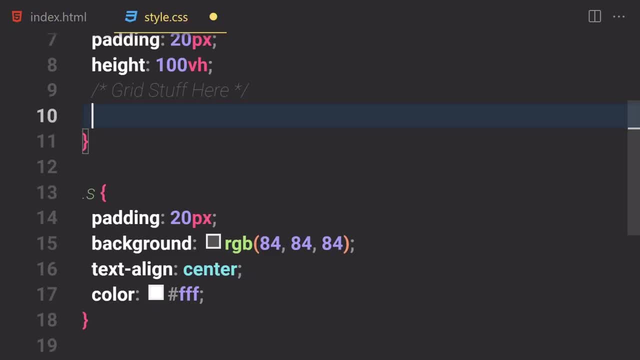 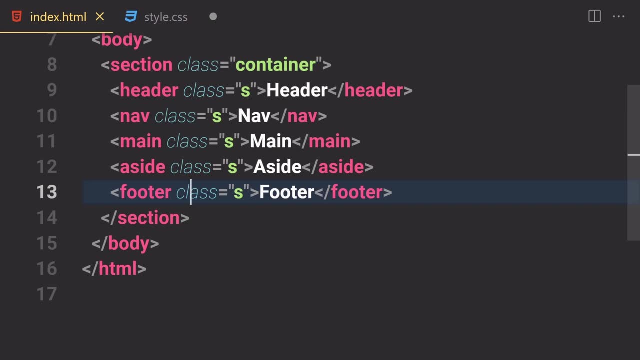 on the container. so the same will goes to the css grid as well. so we have to provide a display grid on this uh container, not on the element. so you just have to remember that. i can't stress that enough. so, first of all, what do we have to do? we have to just write a display. 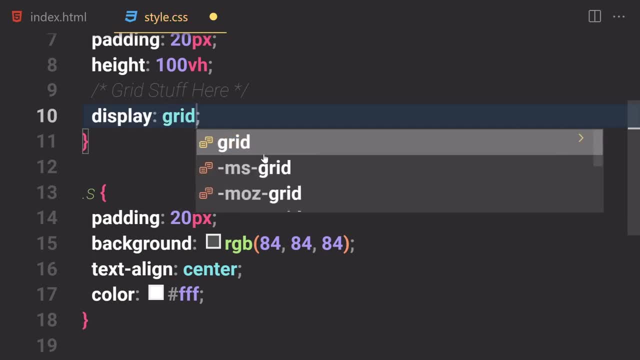 of grid right here. so if you just write a display of grid, the display grid will just define the element as a grid container and it also establishes that a new grid formatting context for our content and all of their html elements. here you can see that they all will become our grid. uh, children. 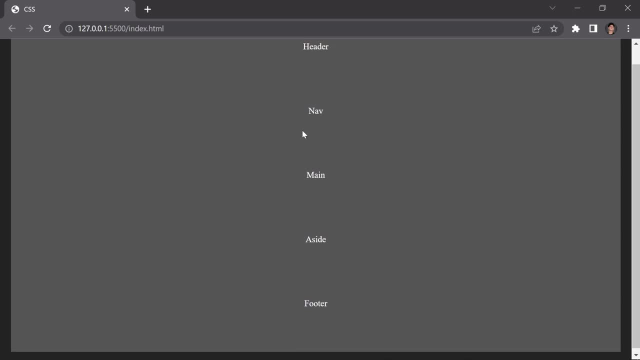 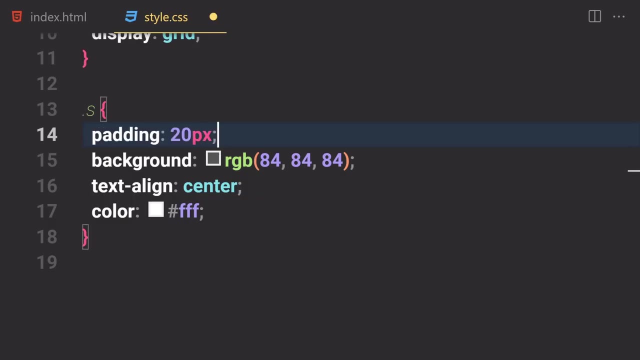 okay, so if you just save that and here you can see, it will now take up all of their entire space. you don't have to worry about that for now, or? you know, i'm going to just comment this padding out. save that. oh no, i guess we are totally cool by that. 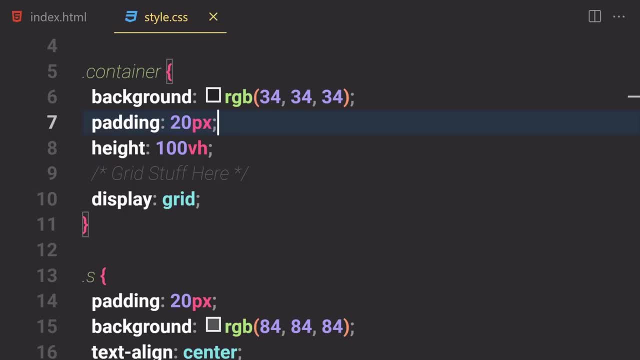 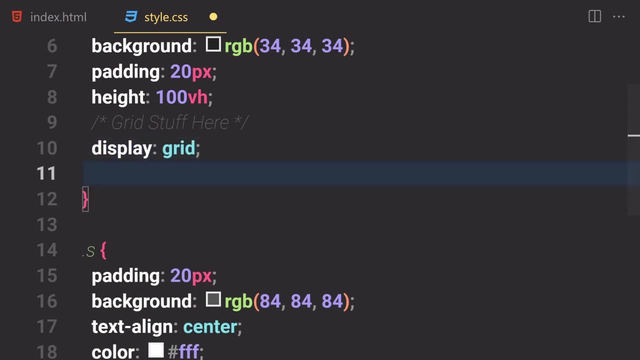 you know, if i just comment this padding out and it will now take up all of the entire area anyway, so let's just write our new stuff. so this is it about a display grid right now. now, the next property which you are going to be learning about is something called a grid. 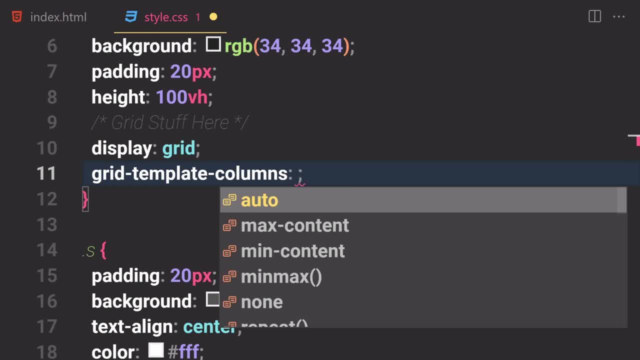 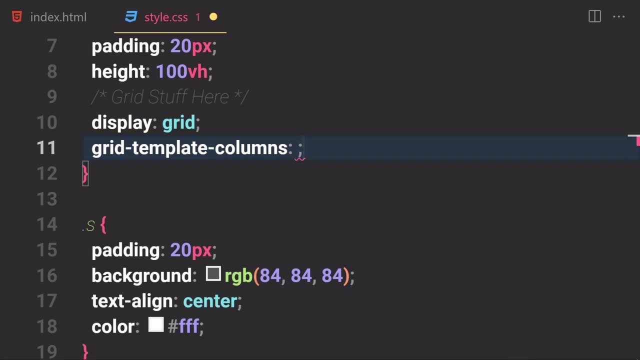 template, uh, columns, okay so. so a grid template columns property specify a number and the width of the column in a grid. okay, so here you can see. we have all of these columns right here. so we have like one column, we have second column, you know what? let me just show you that. 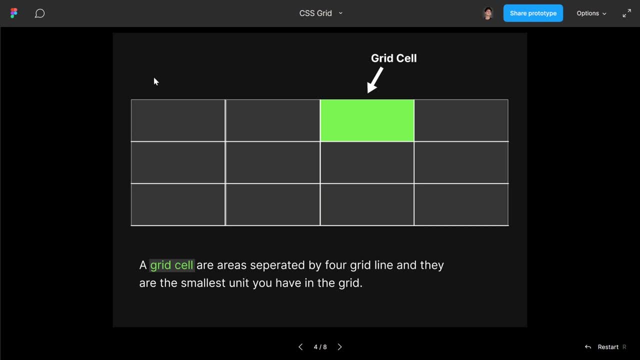 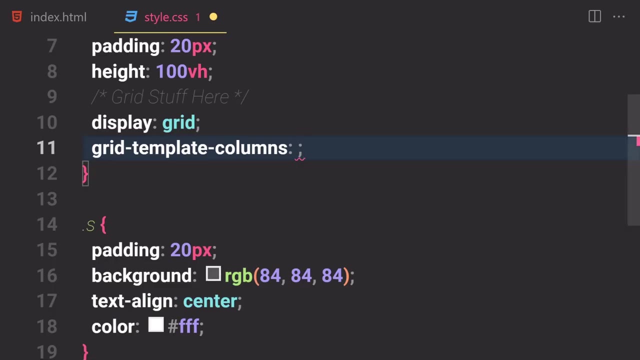 other one. um, i guess that would be fine. so we have that one column, second column, third column and fourth column, and these are rows, like we have one row, second row and third row. okay, so if you want to work with these columns, so for that we just have to write a grid template columns. so what do? 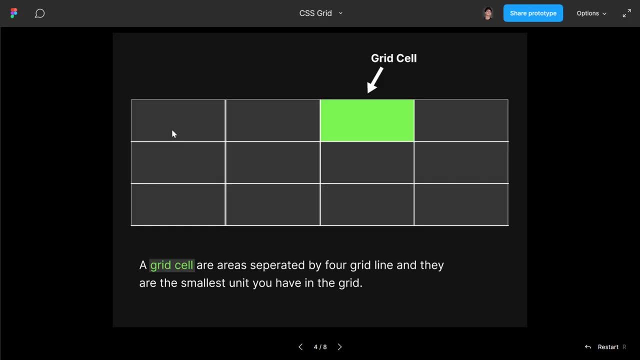 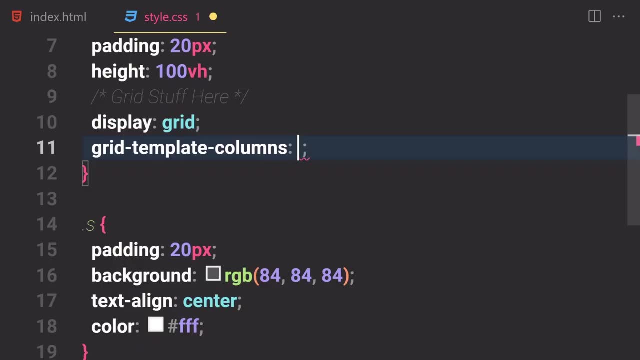 we have to do? first of all, we have to specify the width of that element, like the width of that um columns, and we also have to specify how many we want. so in this case, we are going to be just writing like: maybe, i don't know, i want to just write like 100 pixel, 100 pixel and 100 pixels. so what does all of that even mean? 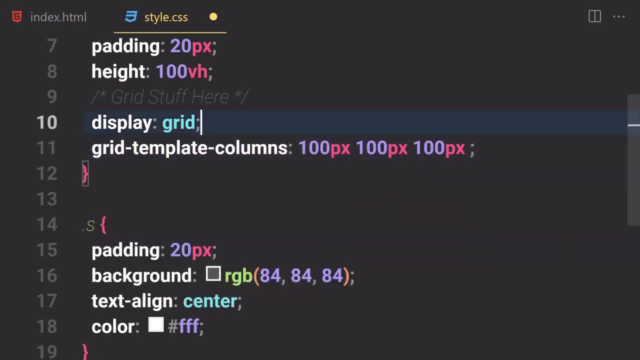 we just write a grid template columns right here and we just specify 100 pixel, 100 pixel and 100 pixel. so it will now give us three columns, like it will give us one column, two column and three column and all of them will have the width and the height of 100 pixels. so if you just save that, 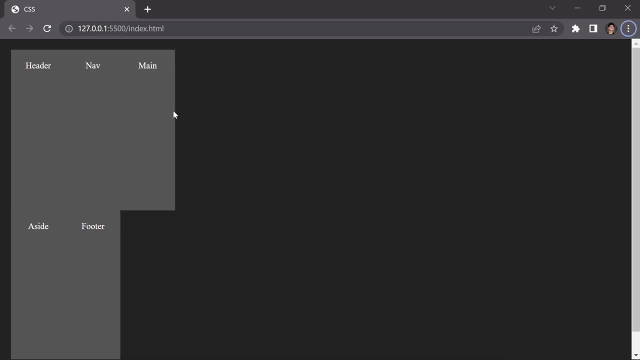 and if you check it out real quickly and i guess- uh sorry, i apologize about that- not the height, but that will give us the width of 100 pixels. okay, so here you can see, we have now three columns. so now you might be asking, like, how is that three? 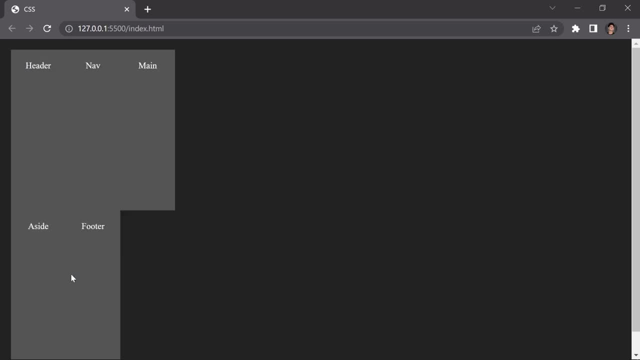 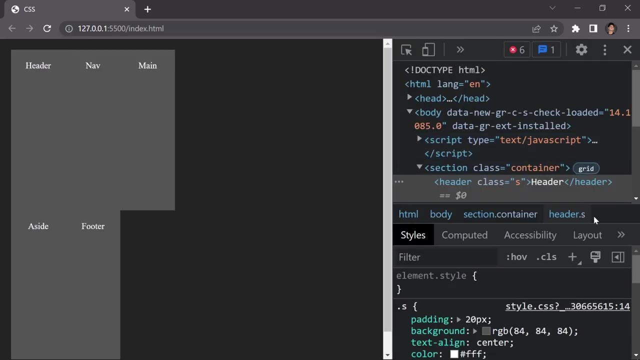 columns. so if you just right click on any of the element and if you click on this inspect area, and now let's just bring that to the left, and now, here you can see, we have this grid pill right here. so if you can see that you have to, uh like, update your browser, and now, in my case, i'm going to just 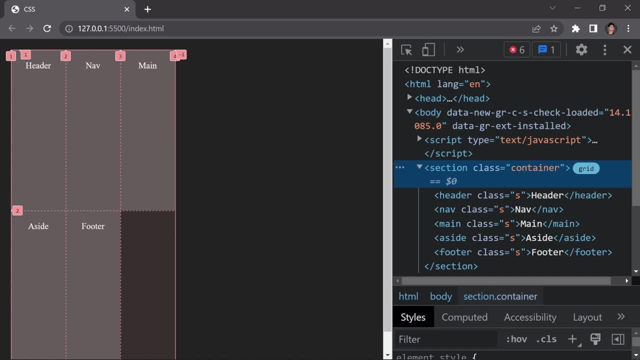 click on that and now here you can see, we have our grid one. i mean like we have column one, column two and column three right here, and i want you to also notice these lines like this, and i'm going to click it in this column here because by default the grid will tell you like i have my line, one line: 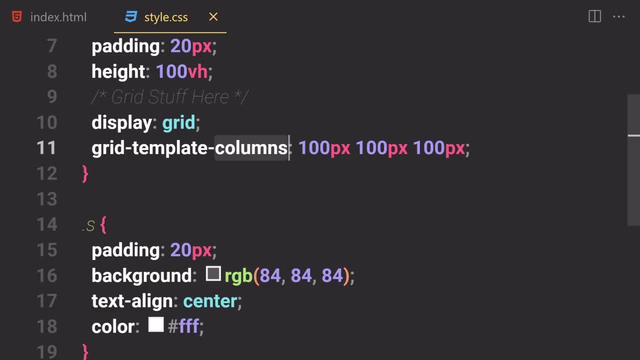 two lines and four lines, and we can't specify the width of the grid. so right now we have the one line, we have three columns right here, and this is how we can specify a different type of column. and now, if you want to provide a different kind of row, so for that we can use property called grid. 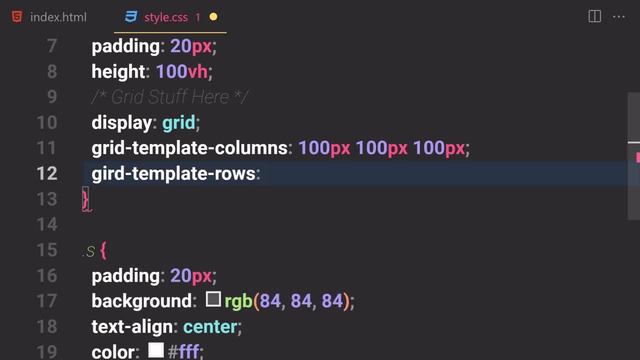 template and then rows, and here we have to specify how many rows we want and what will be the width of that row. so we are going to be just writing like 100 pixels, 100 pixel and 100 pixels. so i guess i messed it up in here. let me just write that one more time: uh, grid. 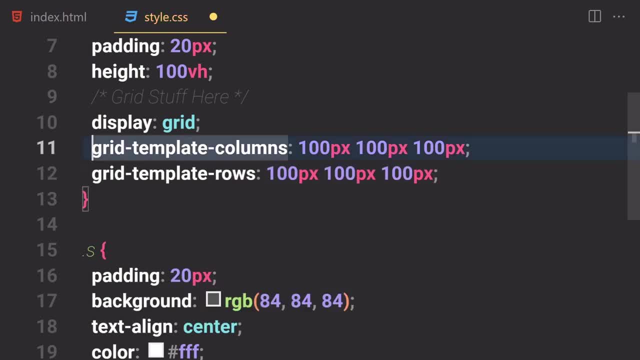 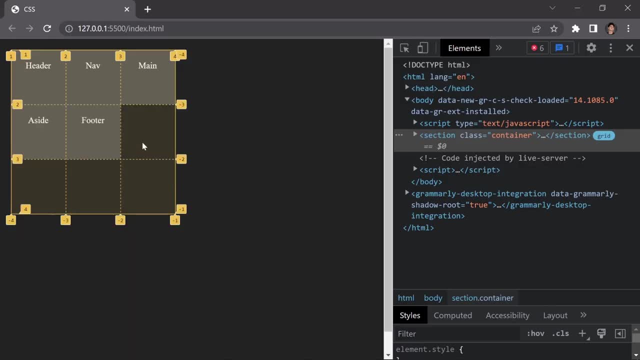 template and rows this one. so we have grid template columns, and then we have a grid template and rows. so guess what will happen? so if you just save our file and now here you can see, it will not use this. three rows right here. so we have row one, row two and row three right here, and we have three. 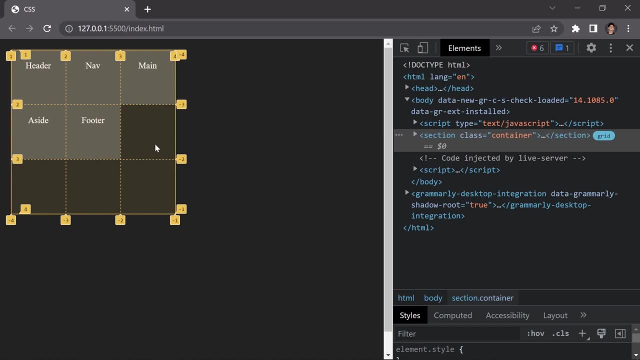 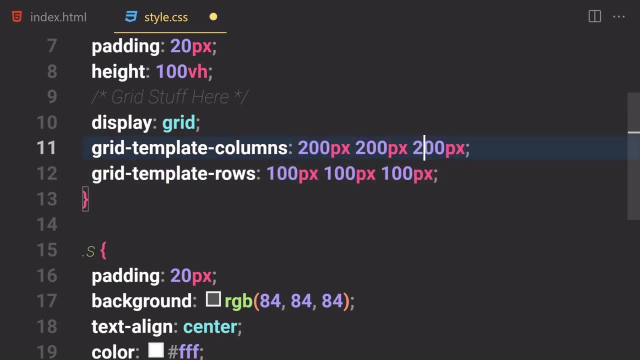 columns as well. so we have column one, column two and column three, and now if you want to increase the sizes of that, so i'm going to just put like 200 pixel in there, 200 pixel in there and 200 pixel in there as well, and if you save that and boom. so here you can see the column sizes will be. 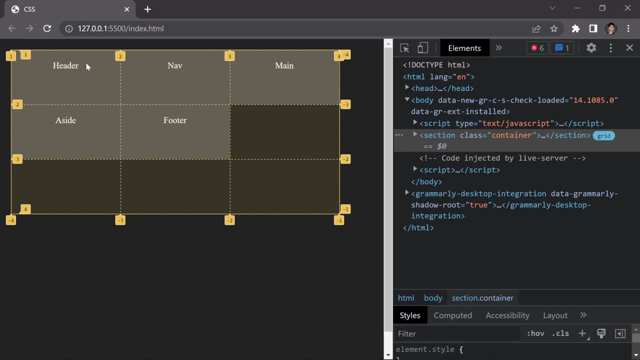 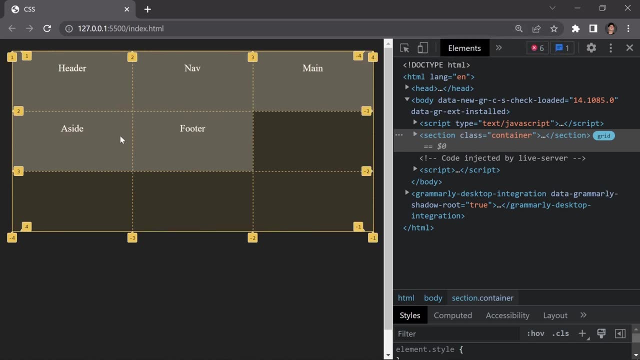 now grow up right here. so we still have that three columns, like we have column one, column two and column three right here, but the sizes are just increased about here. you can see that if you want to increase the size of that row, so for that we have to specify different kind of values to it. so 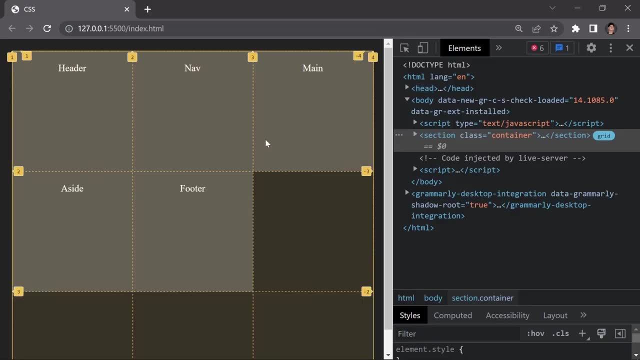 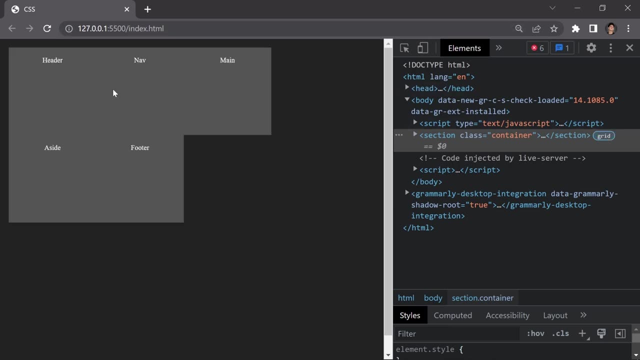 we have 200, 200 and 200. so if you save that and boom, here you can see, it will now just increase the size of that row as well. okay, so if you just uncheck this grid area right here- so here you can see this how currently things looks like- and if you just 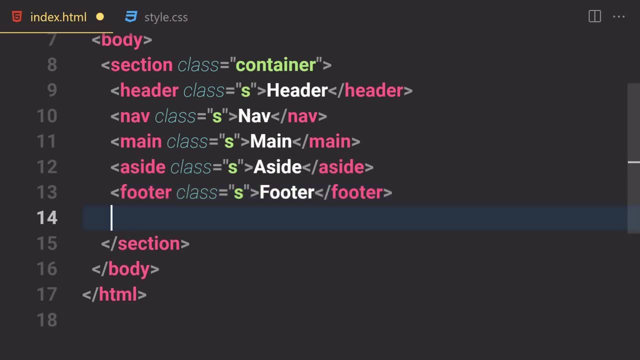 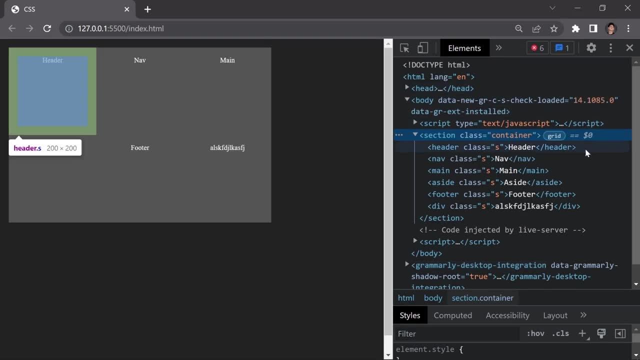 want to provide another last item, so we can also just write like: maybe i don't know, they would be fine with the class of s and we are going to be just writing some gibberish in there and here you can see we are now getting all of that three by three rows and columns, and if you have more, 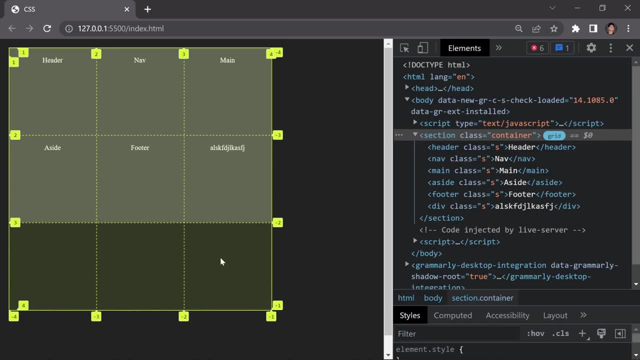 content, and if you have more content, so it will just push it up right here. so these are just a basic properties which you can use for uh, grid. so first of all, we just have to write a. we just have to write a grid. so first of all, we just have to write a grid and we're going to just 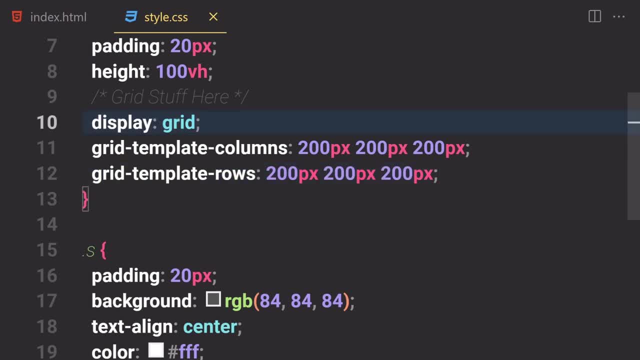 display a grid, so it allows us to work on a grid. and then we have a grid template- columns, and it will allow us to provide different kind of columns to our css or to our layout. then we have a grid template- rows, and it will allows us to provide different kind of rows to our layout. okay, so now. 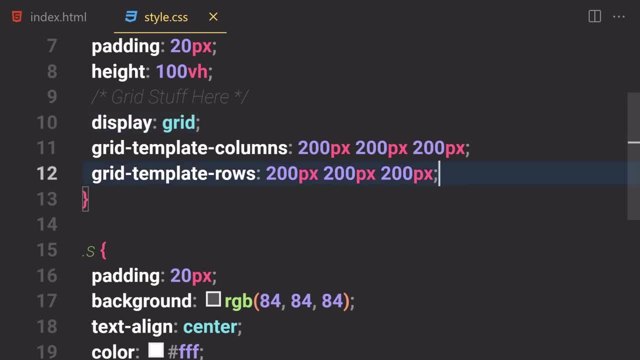 here you might be thinking, like we are repeating ourselves, like we have to write like 200 pixel, 200 pixel, 200 pixel, right there. so for that we can also use something called a repeat function. so let me just remove that real quick, and i'm going to. 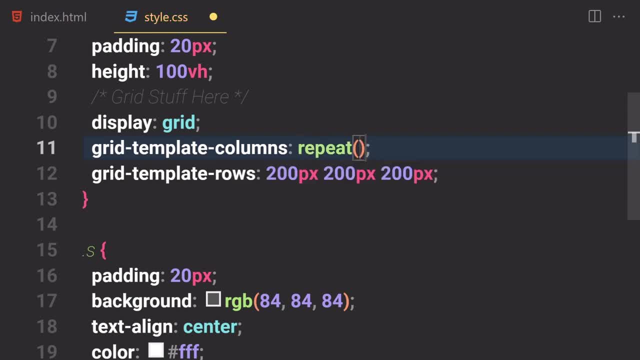 remove that, and here we can use something called a repeat function right here. so first of all you just have to write a repeat keyword and then you have to write your opening parentheses and then closing parentheses. so the first value you have to provide is that how many like columns or how? 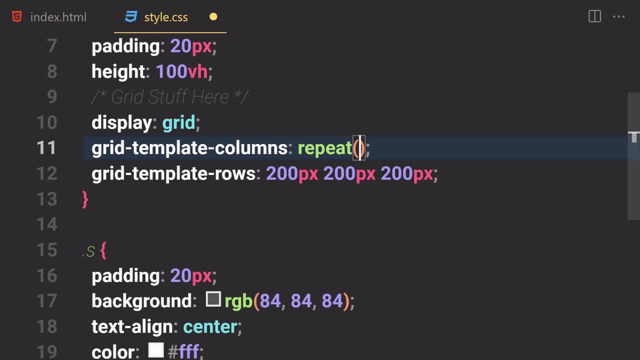 many rows you want. in this case we are working on a column, so in this case, first of all we have to specify how many uh columns you want. so in this case we just want like three, and then you have to specify a comma in there, and then you have to specify. 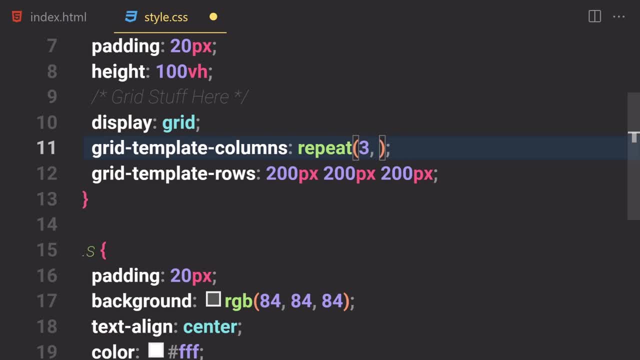 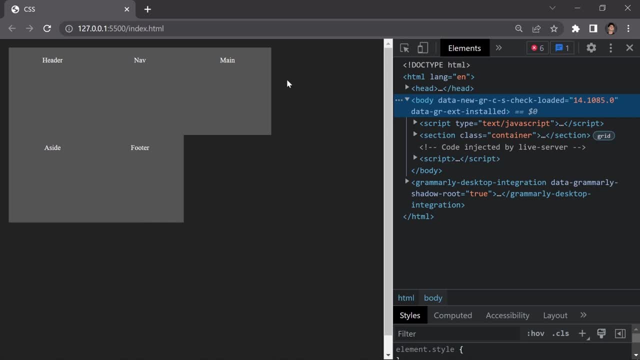 what will be the sizes of that column. so we just have to write like: uh, 200 pixel, and if we save that, and here you can see, that layout will be totally the same. if you want, like maybe, four columns, so we can just change that to four, and if we save that, so it'll also give us one more right. 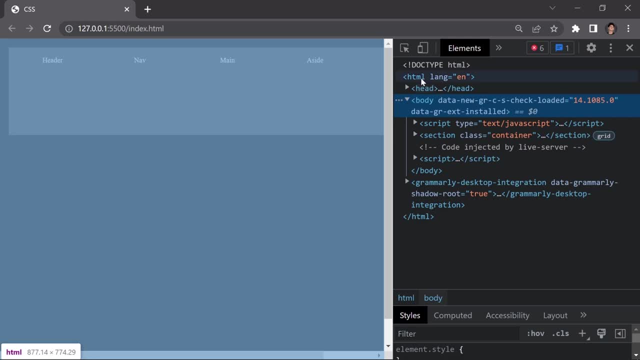 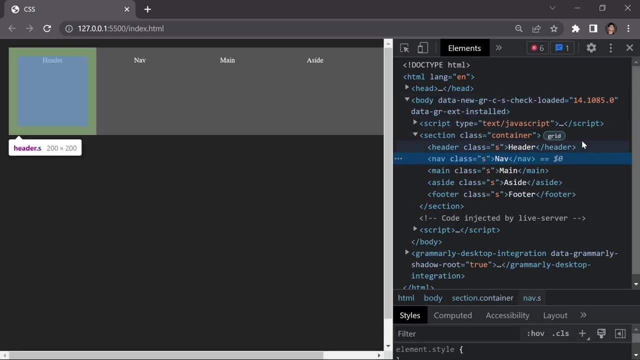 here if you want maybe five of them, and if you save that and it will not give us five column right here, if you right click on there and click on this, inspect okay. so uh, we can also check that out. so if you just click on this grid kind of um. 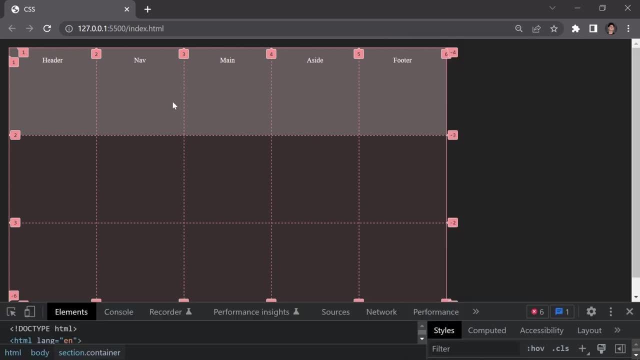 right here and let me just make that here. so, and here you can see, we are now getting five columns. so we have column one, column two, column three, column four and column five. that's because of that function which we use right here, so we are going to be just setting that to three right here. 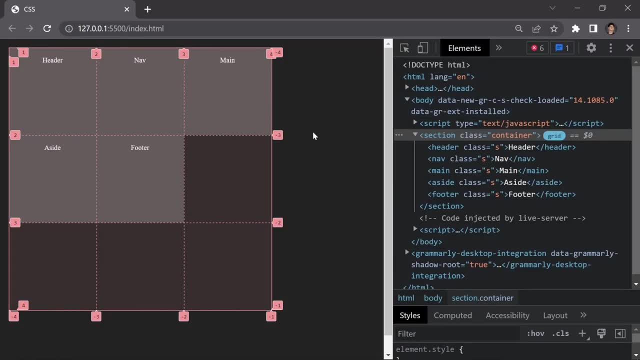 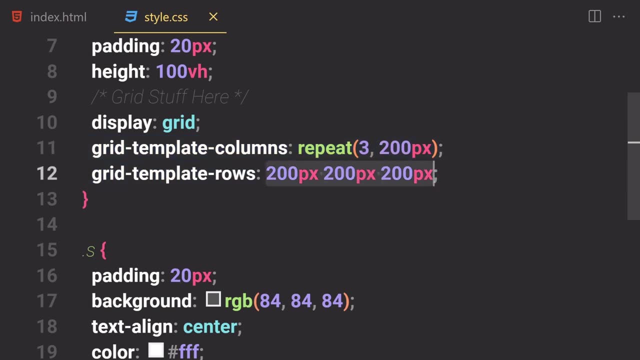 and if we save that, it will now gives us three columns right here and we can also use that same repeat function for these template rows. okay, so if you just remove that, instead of writing like 200 pixel, 200 pixel and 200 pixel, we can use this repeat function. 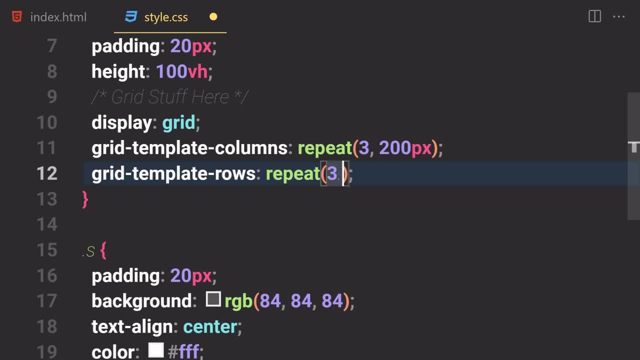 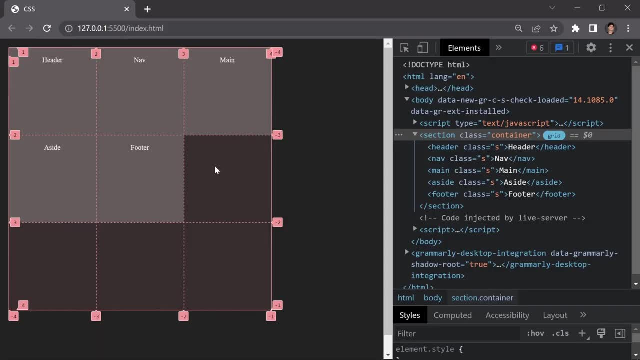 so we can also use this repeat function. first of all you have to specify how many you want and then you have to specify the sizes of that. like in my case, i'm going to just write like 200 pixel, and if you save our file and boom, everything is looking the same as before. okay, so we can also. 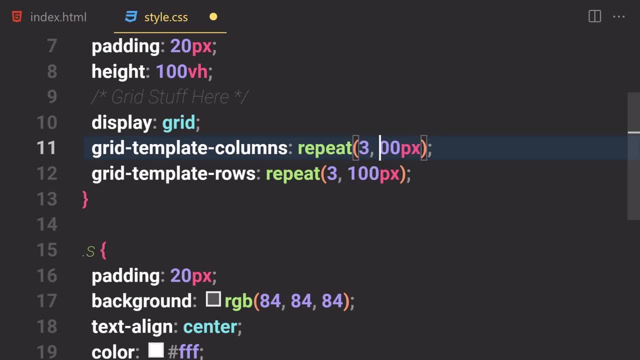 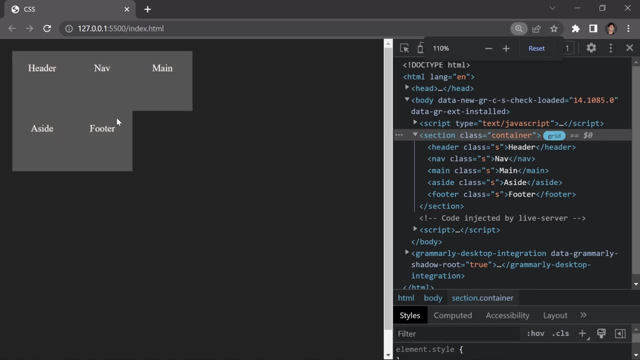 increase or decrease that if you want to. so like, instead of writing 200 pixel, we can also set that 200 pixel, if you want to, and if you save that. and here you can see, now our grid is kind of small. that's because we make our elements or our items a little bit small, okay, 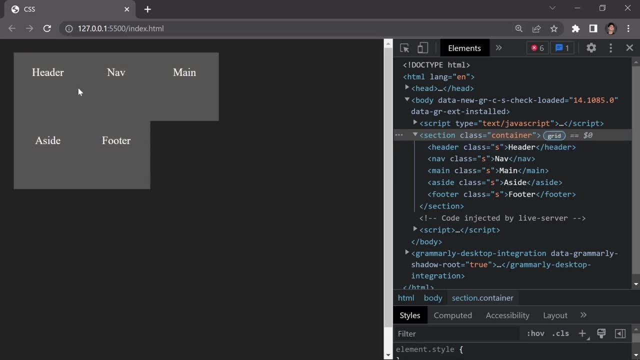 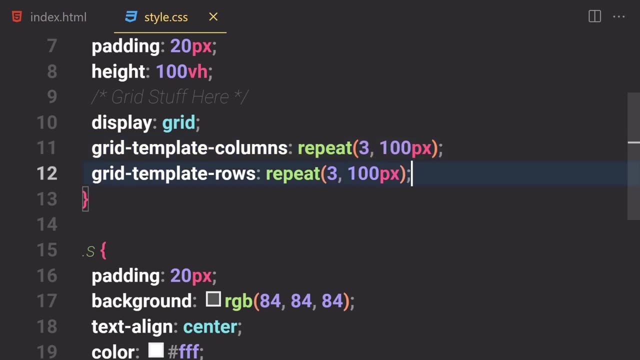 this is how everything looks like. and now you might be thinking like we can also provide a little bit of margins so that we can separate our item. but for grid you're not going to be using any margin and stuff. for grid we use something called a grid. uh, let me just write like a gr. 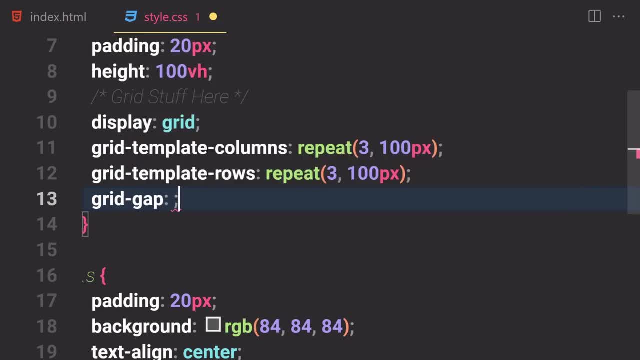 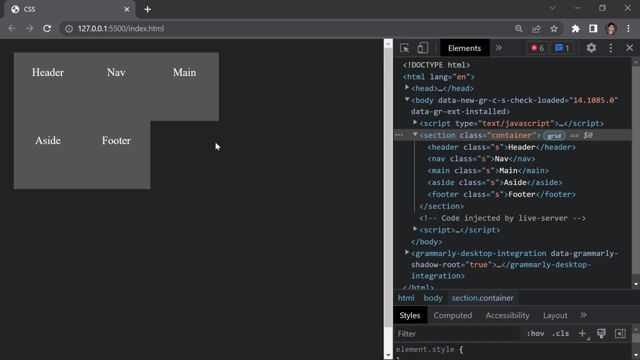 gr id and then gap. so we use this grid gap property and it allows us to provide a gutters, and a gutter is just a space between each lines or each row or column, whatever you want to call it, and we can specify a grid gap for a row. 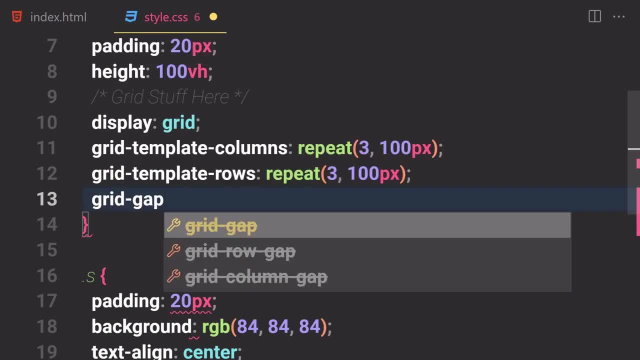 as well. so for that we have to just write like a grid gap to the row. i guess it was like a grid row gap, i'm not sure. yeah, no, it's not a grid row gap, i'm not sure, but we are not going to be using any of that and you won't need that. but that was just a long way, right, or? grid gap. 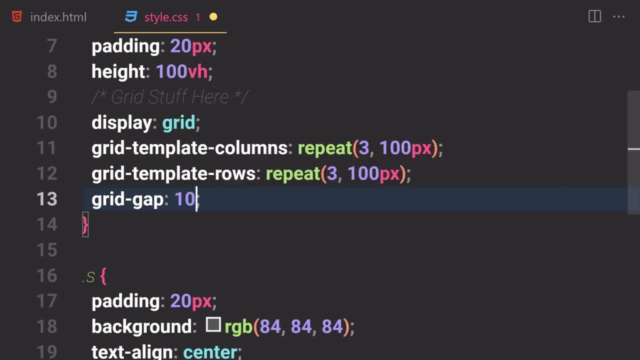 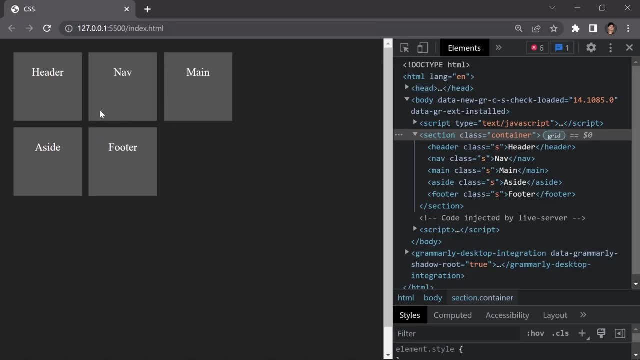 but in this case we are going to be just using a grid gap right here and we have to specify how much the gap you want inside each of the element or each of the cell. and if we sell that, and here you can see, run log uses 10 pixel of gap right here in each element. so this is. 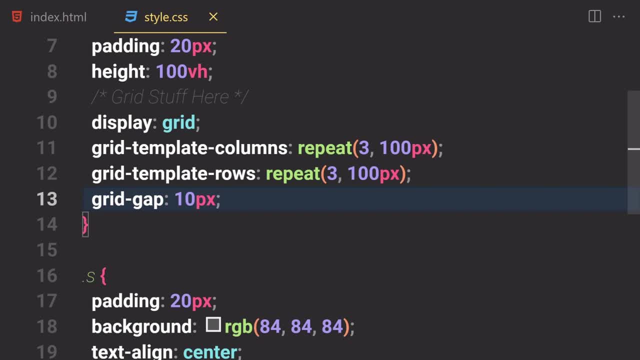 kind of simple. so so now that we learned about four properties in css grid, and now let's just learn about something called a fr, and fr stand for a fractional unit. you can learn more about that, but my recommendation will be to do not waste a lot of your time on that. first of all, let me just 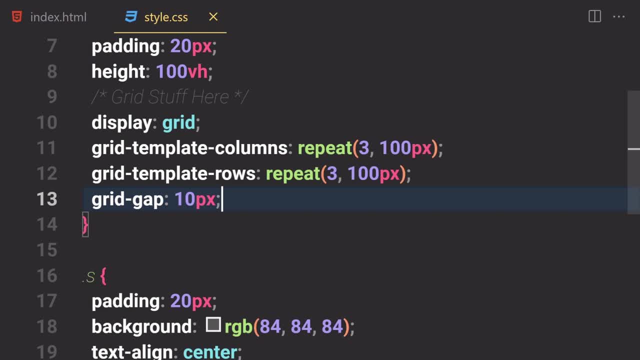 give you the definition of it. so, uh, so the fraction unit is an input that automatically calculates the layout division when adjusting for a gap inside the grid. so that was just a definition of, uh, what do we call it: fr unit or a fraction unit? let me just say that one more time. so the fr or the fraction unit is an input that automatically 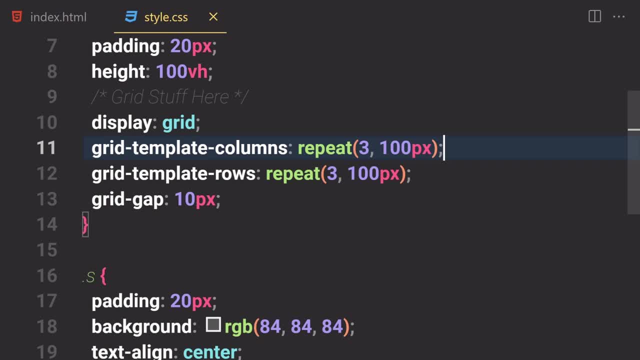 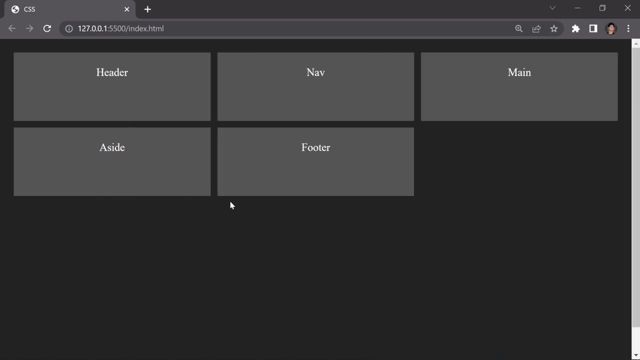 calculates the layout division when adjusting for the gaps inside the grid. so instead of writing like uh, 100 and 100, we can write one fr, and this is very powerful. so if you just use like one fr right here and if you save a file and boom, here you can see, it will now just take up all of the. 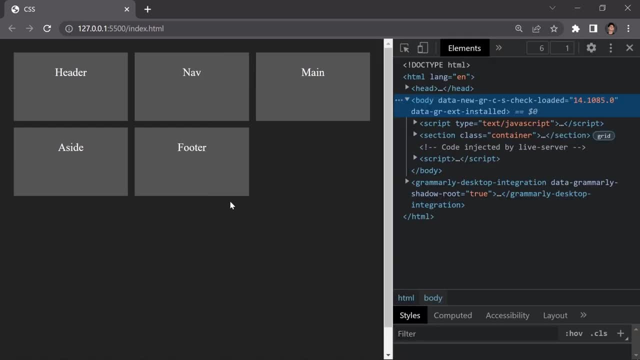 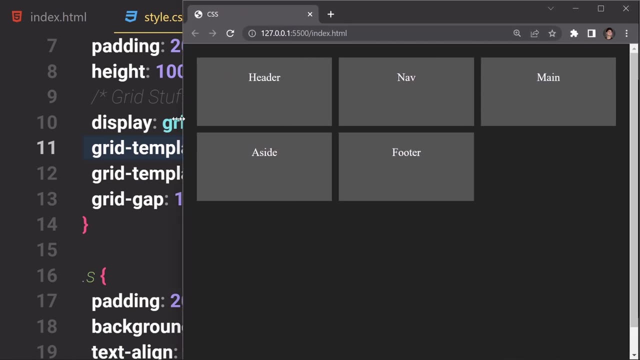 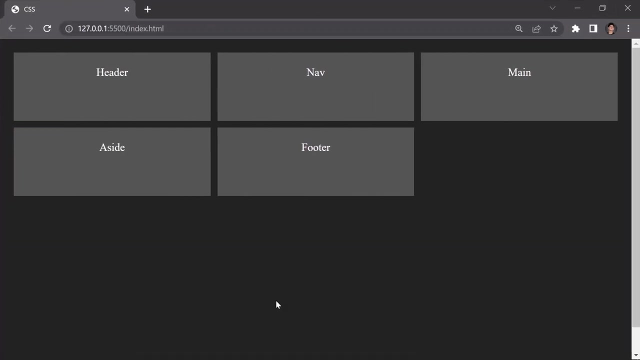 entire space, depending upon the screen size. so if you just make that like bigger or smaller, so here it will also shrunk down the elements, or it will also make it bigger like so okay, so here you can see everything. so this is the fr unit. you can use like um fr unit if you want to, or you can just use 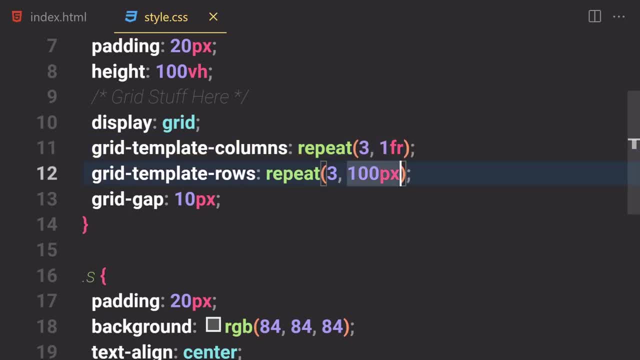 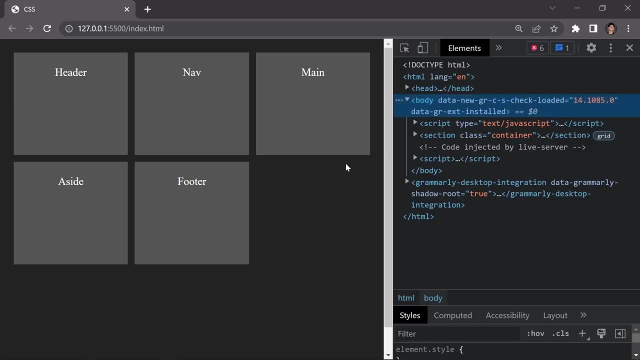 a pixels, but i just kind of want to show you the fr unit as well, and we can also use it for a heart as well. so if you save that and boom, so we can also use it for rows as well. so that was it about for fr unit or fraction unit, and we learned enough about the css grid, so now let's just learn about. 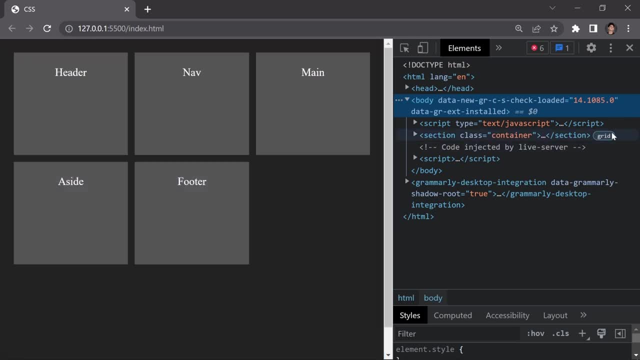 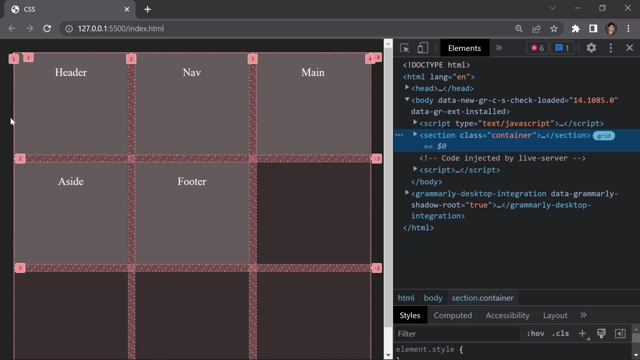 the css grid. so now, in this case, if you just click on the css grid right here, so here you can see, we have our first line, or our first line will start out from here. so this is going to be our first line. then we have our second line right here. so now, if you want to span this element like: 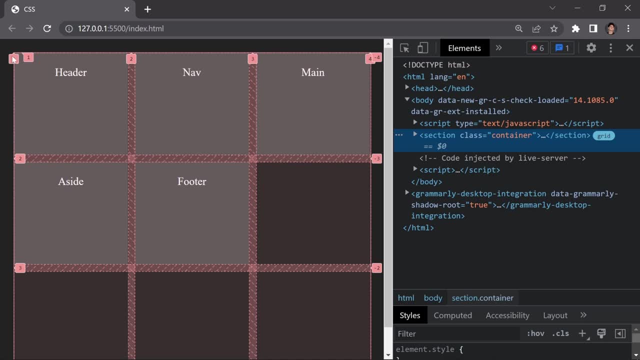 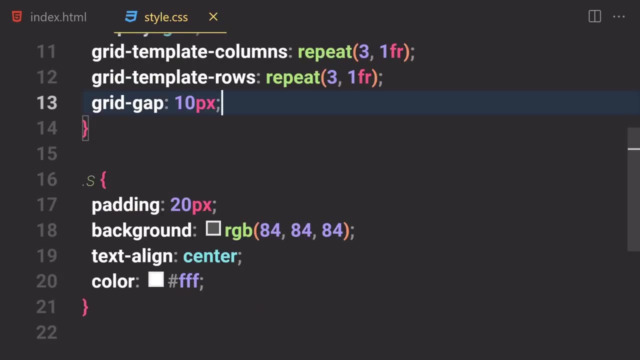 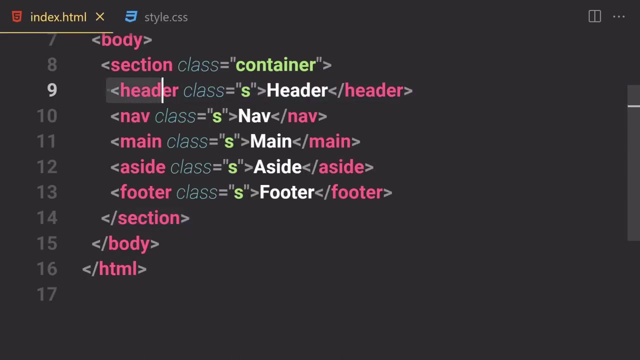 this h1- not h1, but this header area- to span from this grid line one to this grid line three. so we can also do that by using a grid uh properties. so let's just learn about that. so if you want to work with this grid line one element, for that we have to select that specific element. so, like if you: 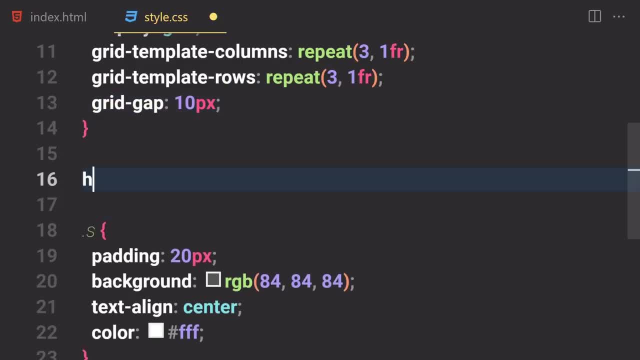 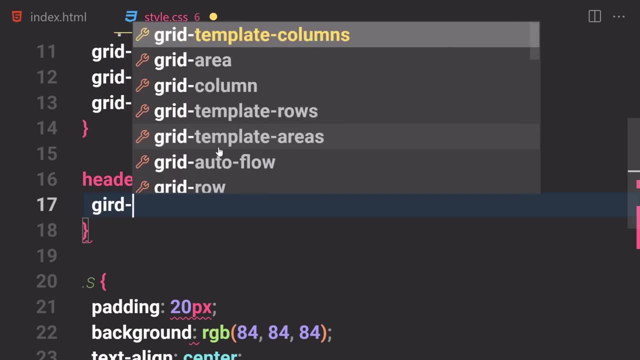 want to spend this header. first of all, we have to select that. so we are going to be first of all selecting this header, right here and now. what do we have to do? we are going to be using something called a grid and then column. in this case, we are spanning a grid column and we can also go with a. 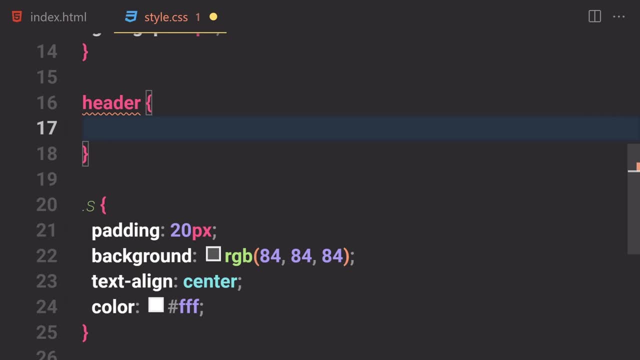 longer way. first of all, let me just show you the longer way, and then i'm going to show you the shorter way. so i'm going to just write like grid column and then start: so where do you want your line spanning to be start from? so i'm going to just provide like one, and here you can see we are. 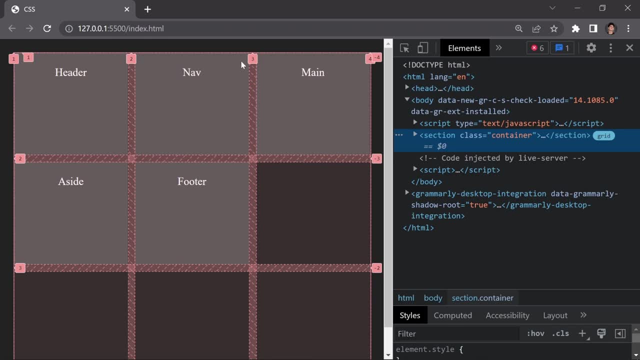 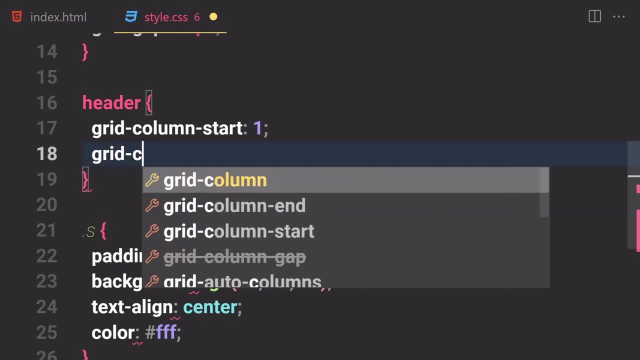 now, starting from this one right here, and we want to go to this third line right here. so for that we have a new property, not a new- i shouldn't have to say new- but for that we have another property, grid column, and then n, and now if you want to span or element, and now if you want to. 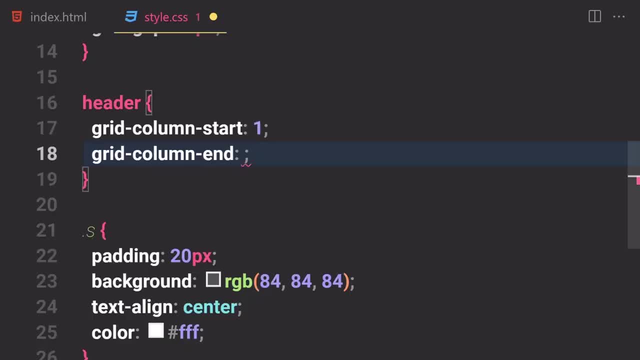 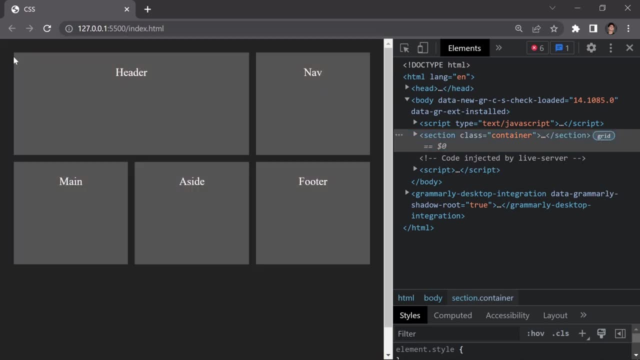 span or element from this one line to this third line. so for that we can just provide a three right here and now. if we save that- and here you can see if i just uncomment or uncheck this grid right here- so it will now take all of these three lines, so it will now spin from this item like from: 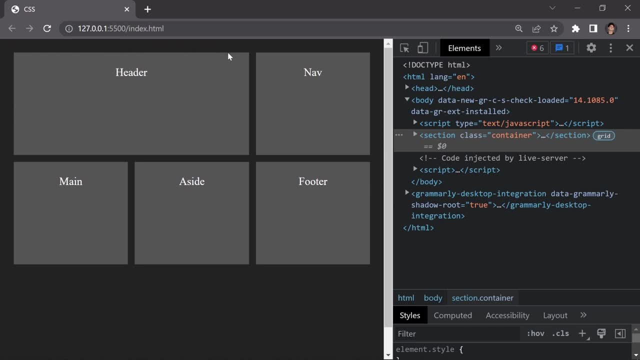 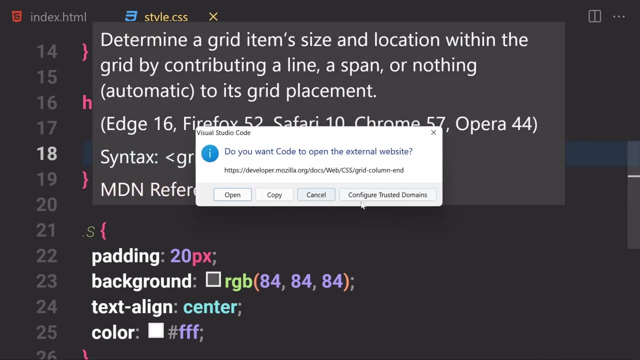 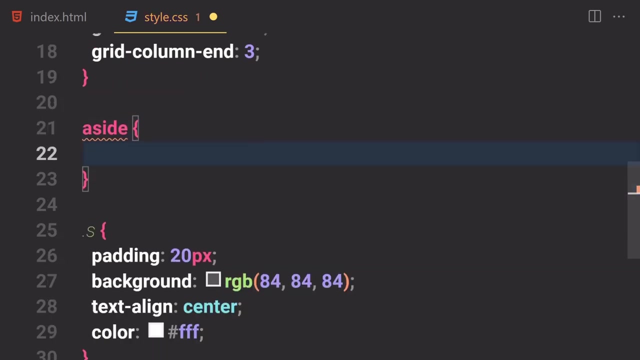 this grid line one, to this grid line two and finally to this grid line three. okay, so we can also spin around this aside, if you want to. so for that we have to first of all select that aside. so let me just select that aside aside, right here and now. let's just provide our grid column. 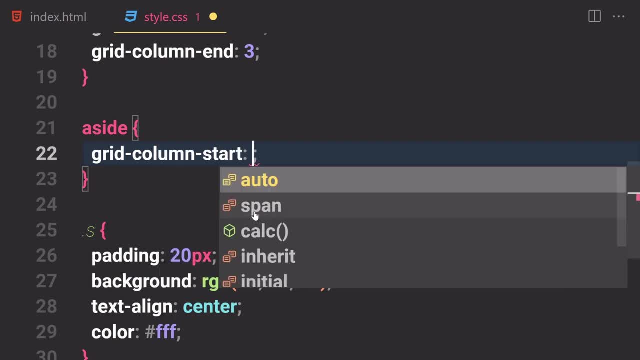 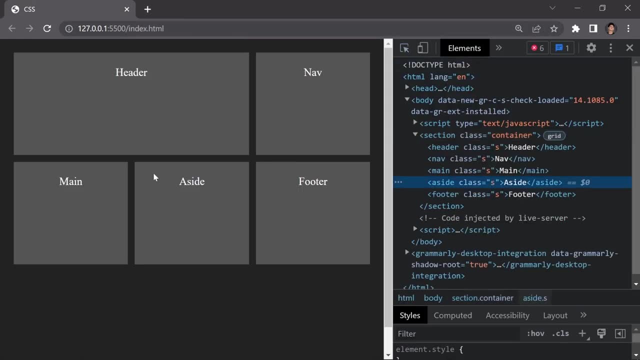 or yeah, grid column will be fine, so grid column start. so you want to start from the line. so if you just try to click on that- and i guess i'm going to just click on this aside right here- and let's just select our container, let's select work and grid, right here. so you're going. 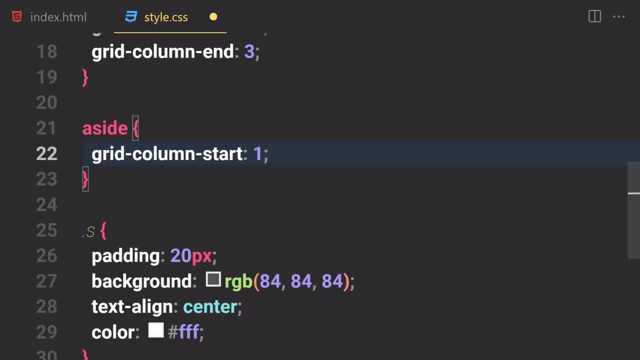 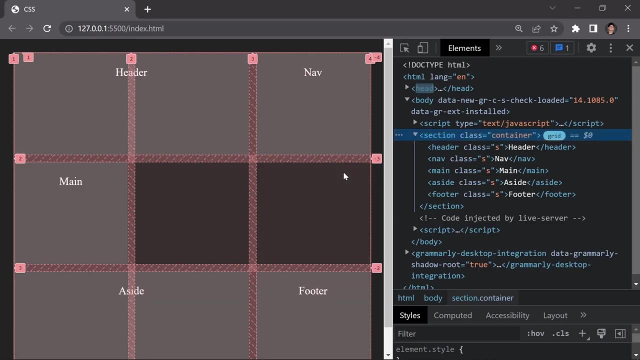 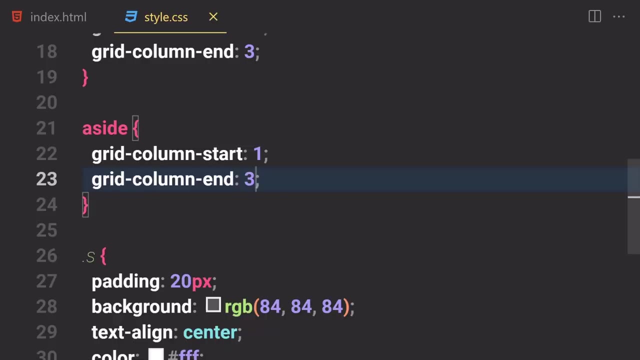 to be writing a grid line of, i guess one would be fine. and now if you just write like a grid column and then n and we want to end it through the third one, so if you save that and it will now push our item to a new line because we don't have any space for that. so this is how we can spend our element. 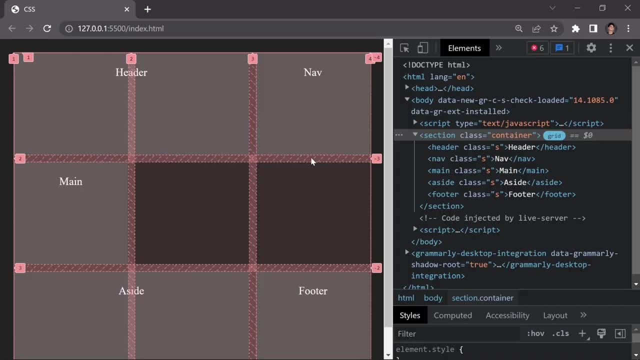 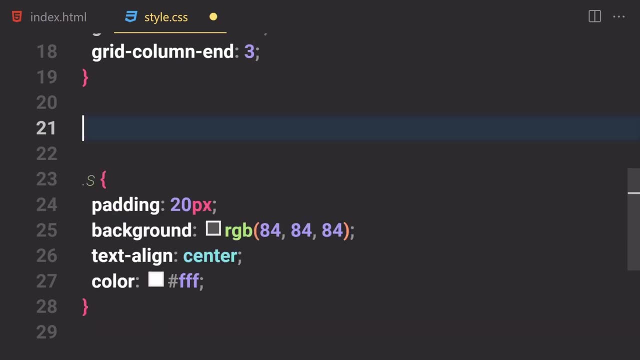 or you know what. we can just write it from like second item to the third one, and if you save that and there's the default behavior, that's the default behavior. we shouldn't have to use that. so i'm going to just remove that. and now let me just show you the shorthand for writing a grid. 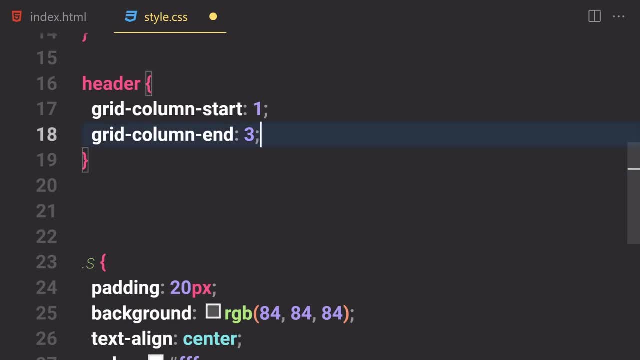 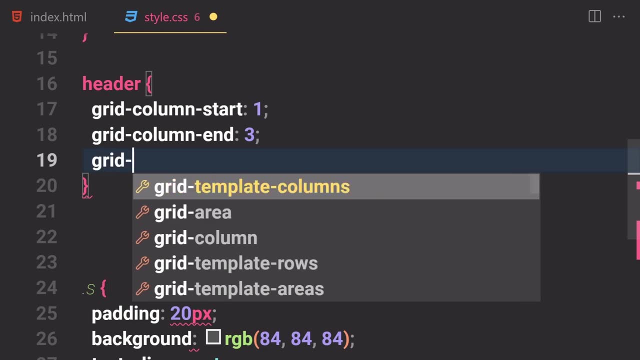 column start and grid column end. and, by the way, i'm going to also show you, uh, a grid row start and grid row end, and then i'm going to show you the shorthand for that. so i'm going to just write, like a grid, a row and then start. so now, in this case, uh, first of all, we just learned about how to. 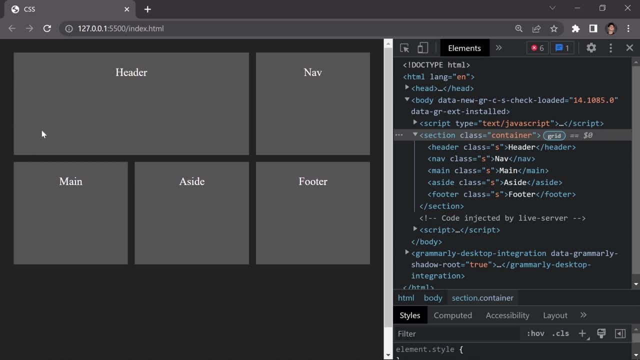 we can spend our item by using a column. so we can also spend our item by using a rows. so you know what i'm going to comment both of these lines out and if you save that, and this is how, by default, our elements looks like. but now, if you want to start from this line and you want to go through, 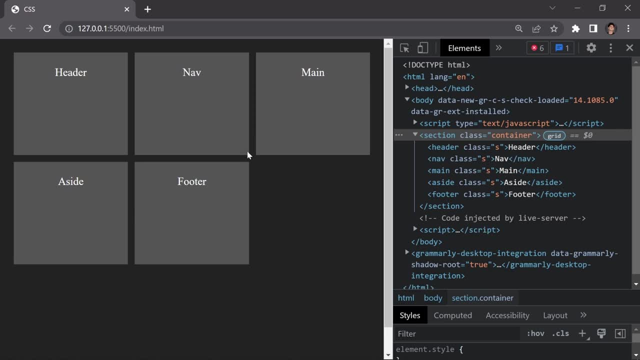 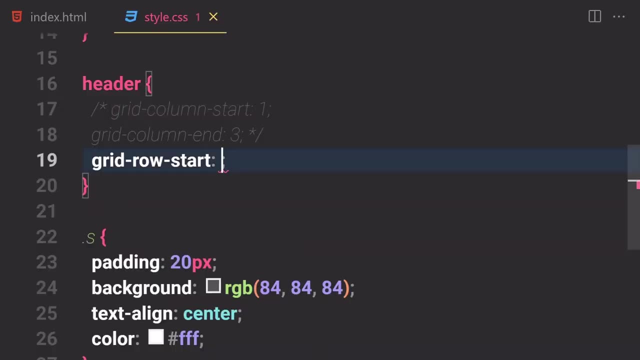 this element. so like, if you want to spend from this line one through this line, uh three, so yeah, we can also do that by using our grid row star property. so we are going to be just specifying one right here and now. let's just use like grid row and. 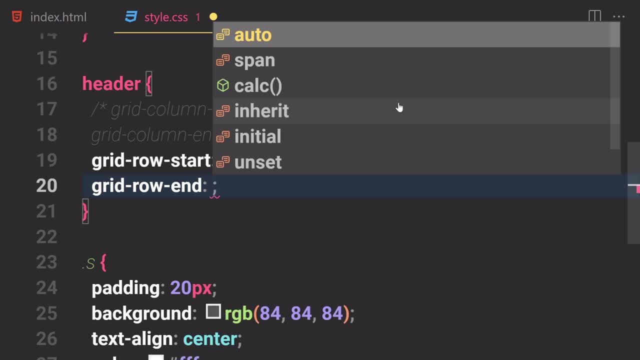 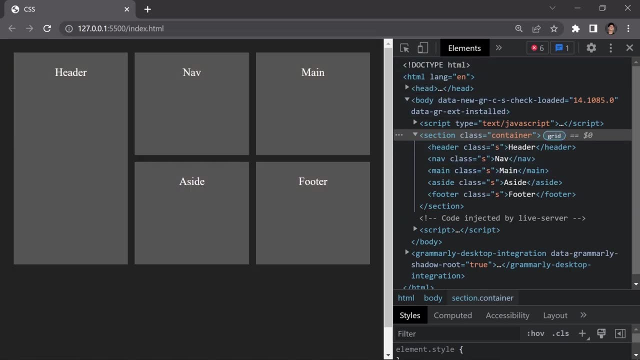 then n, and here we have to specify: where do you want to end, or spanning, so we can just provide three, and if we save that and boom, so i guess- yep, that's what's going on, and here you can see- it will now span or element from that line one through this line three, right here. okay, 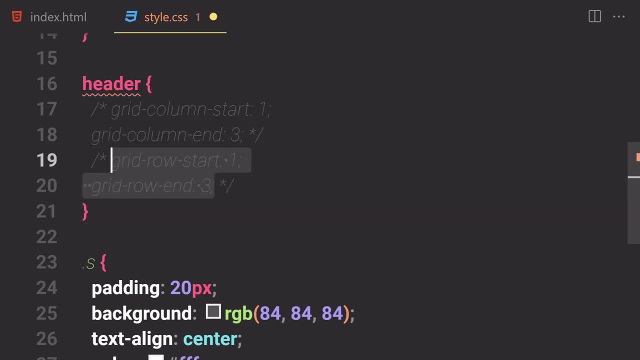 so we can also use a shorthand for that. first of all, let's just comment these out. first of all, let's just learn about the column one. so we are going to be just using like a grid column instead of writing a grid column. start and grid column and we can just write like a grid. 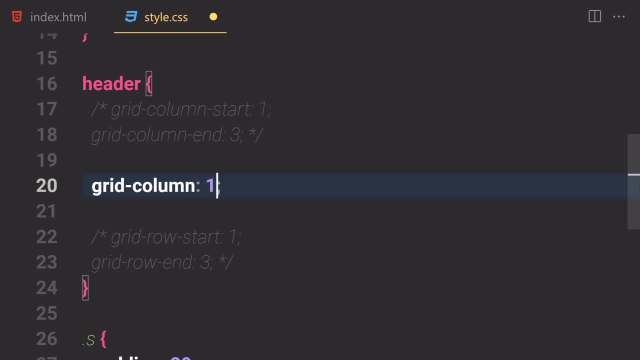 column, and here we have to just specify where do you want to start, or grid line, and then we have to specify a slash and where do you want to spin through. and here we just have to write like three right here, and if you save that and here you can see, it will now just start, or spanning from this. 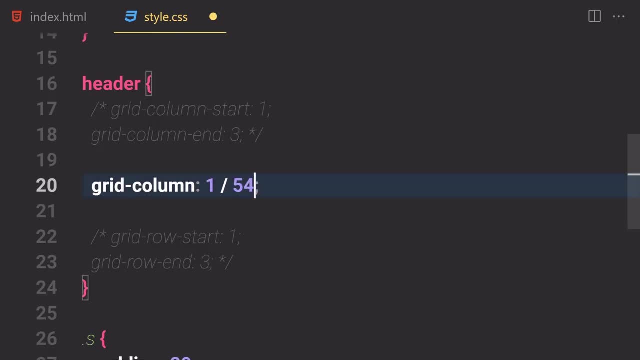 first area to this third area, and we can also spend through like four if you want to. so if you just write four and save that and here you can see, it will now just spin through like so and we can also use a shorthand for this grid row. start in this grid row. 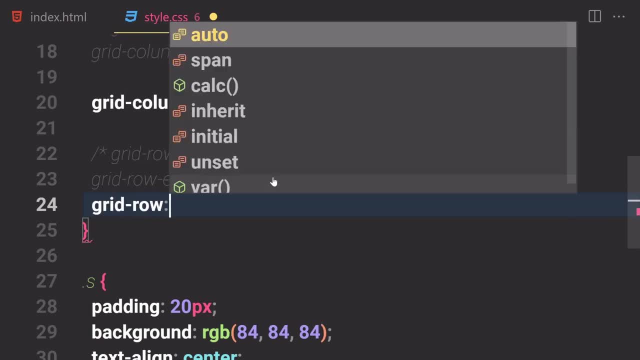 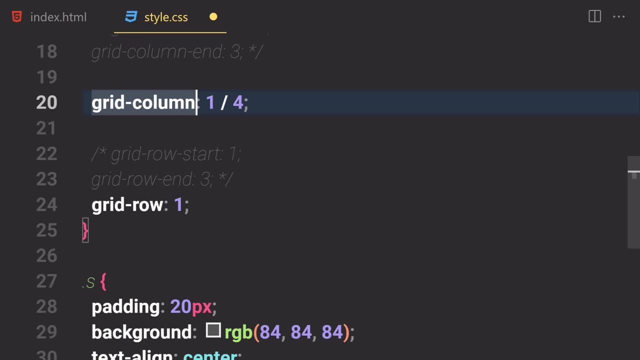 so we can just write like grid row and then not start and end. but we can just provide like a grid row right here and first of all we have to specify where our element should start. first of all let me just comment this line out: where our element should start, and then we have to specify the. 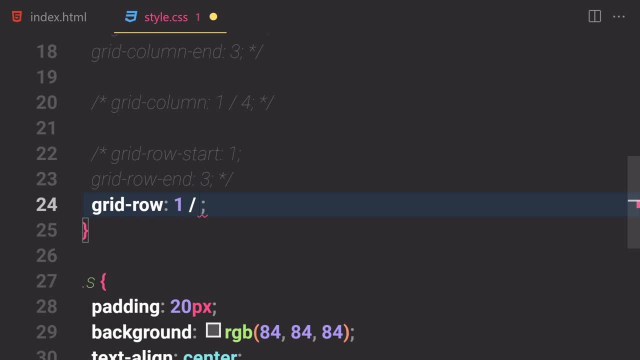 slash and then we have to specify the value for, like, where our grid spanning should end. so we can just specify like three right here, and if we save that, and boom, and this is how it looks like we can also write four if you want to, and it will now just spin out: okay, like that. 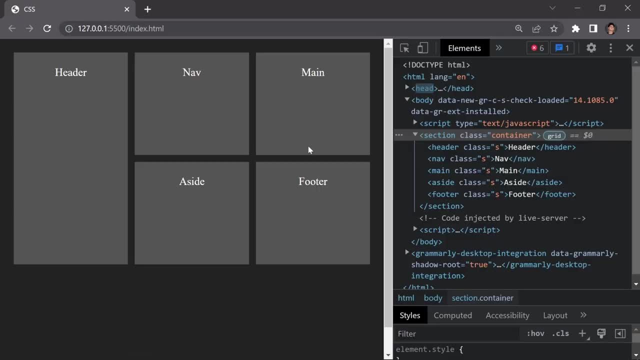 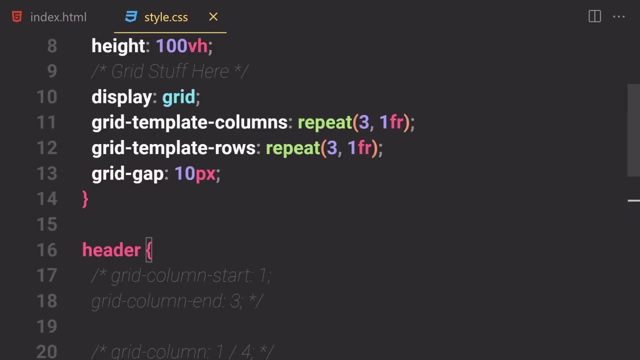 we don't want that, so we can just go to like third one and this: how everything should work anyway. so this is just a little bit about display, grid template column and template rows, then grid gap. we also learn about repeat function. we also learn about something called a grid column start. 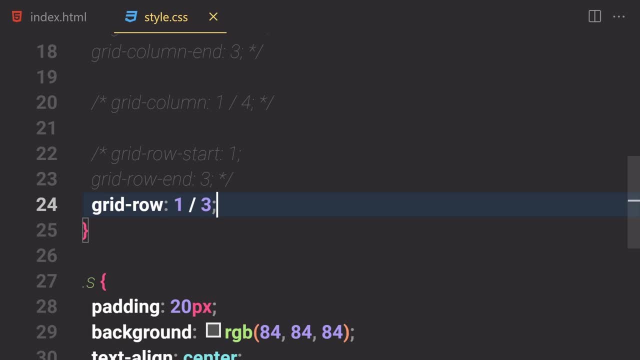 and end and grid row start in end, and we also learn about a grid column and grid row. so now let's learn a little bit about the grid naming, like we can also name or grid line if you want to. so for that, you know what. i'm going to remove all of this, and i'm going to remove all of this. 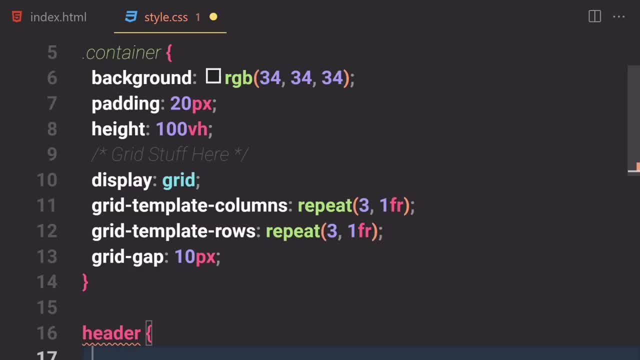 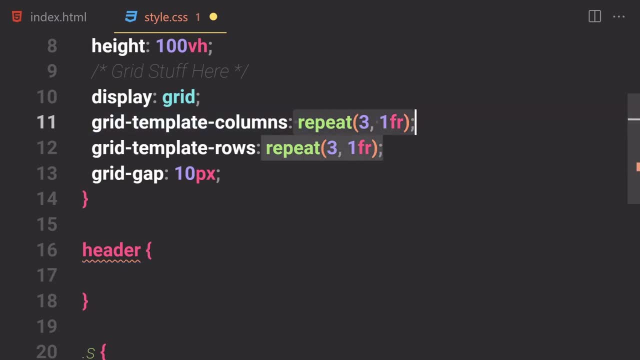 coding right here. so i'm going to just remove that. and now here we can also give a name toward element. but if you want to name or element or line, to be precise, for that we don't have to use these repeat function. so i'm going to remove that and instead i'm going to just 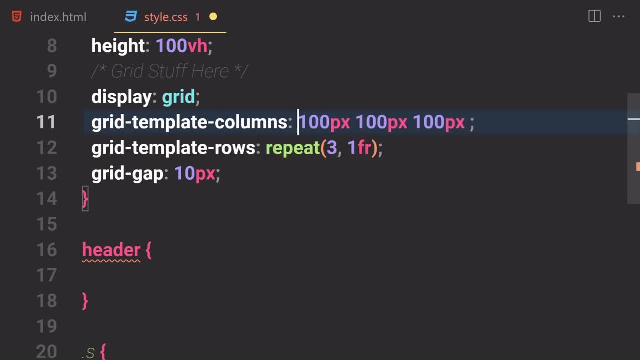 write like 100 pixel, 100 pixel and 100 pixel, so we can also name our first line to be like. and by the way, if you want to name your element, first of all you have to write your opening bracket and then the closing bracket. it's not parenthesis like these, it's not parentheses and. 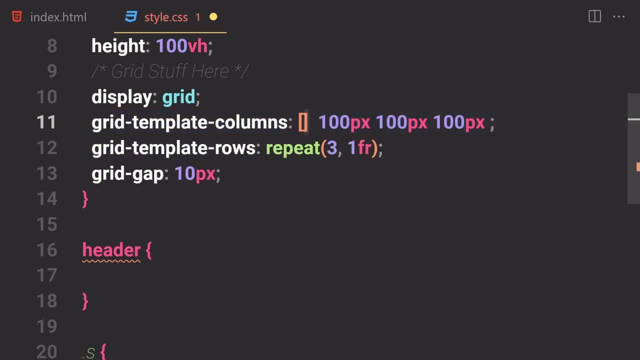 not a curly braces. these are opening bracket and closing bracket right here. okay, so here you have to specify which kind of name you want to give to your first line. so in this case, i'm going to just write like: uh, i don't know, i'm going to provide like a start in here, a lowercase start. i'm going 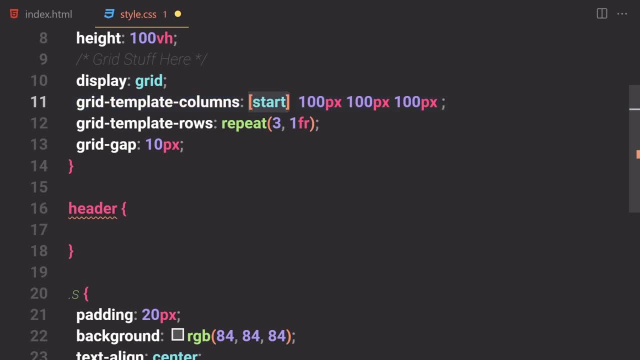 to zoom out a bit. so this is going to be the first name for our line, and now let's just put: uh, maybe i'm going to name this one, so i'm going to just put our second bracket in there, and here we just have to specify the name for that, like in my case, i'm going to put like n, so that is going to be the. 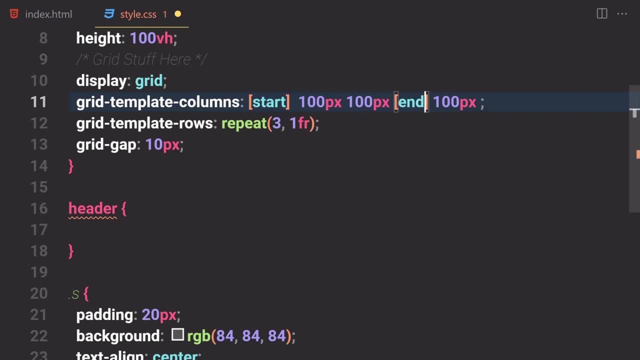 default behavior. i guess you know what we now. we are totally name or lines, so now let's just span through by using these lines. so i know this stuff can be a little bit confusing and it's not that much useful either. like you will just find yourself a little bit, like you may or might use this. 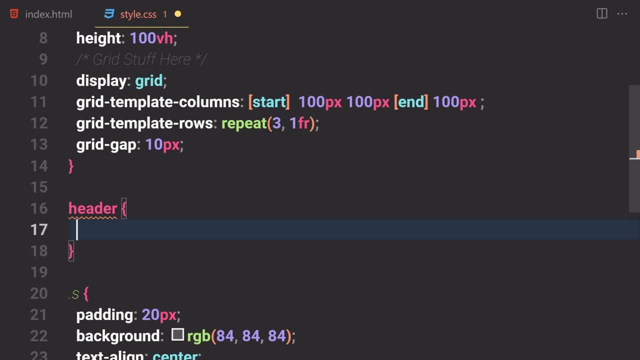 naming or not. i can't say that for sure, like i guess i can't guarantee that you would use that naming that much often. but if you want to you in your project and you want to be looking a bit cool so you can name your line if you want to. 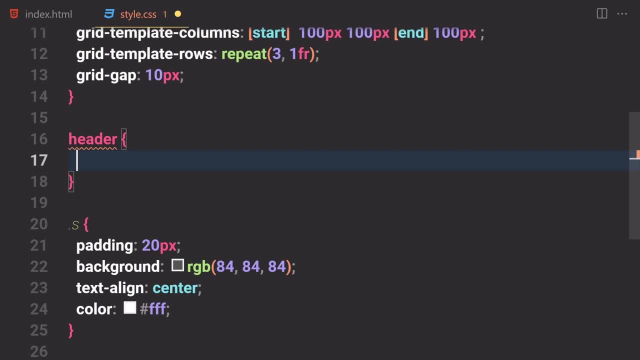 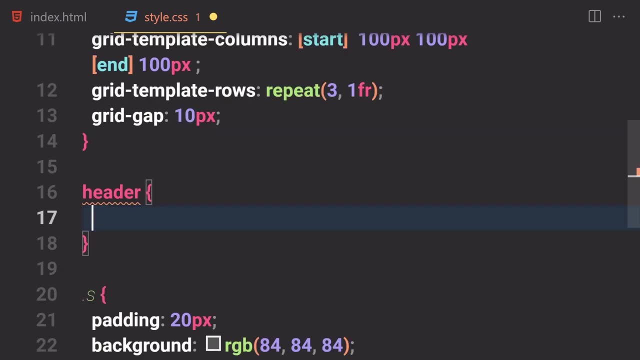 but i just want to put it in my course, because this is a complete guide. so now there will line or lines, like we have started, and and right here. so now let's just span through that, so we can just use our grid column, and here we just have to specify where we want to start, or spanning. so 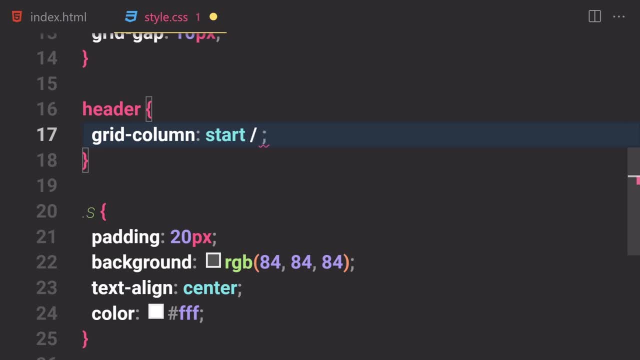 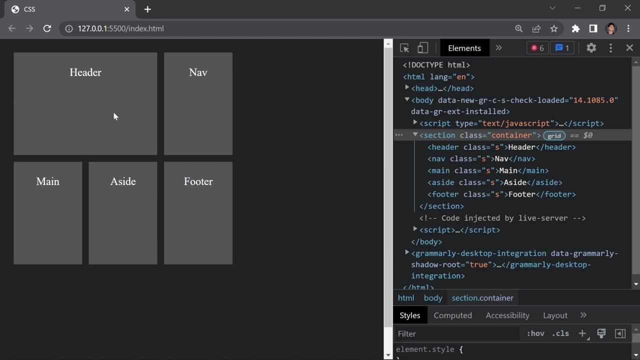 we can just write a start right here and where do you want to end your spanning? so we can just end it to the end. and if you save that and boom here you can see it will now just take up the second element right here and we can also take up the third one as well. 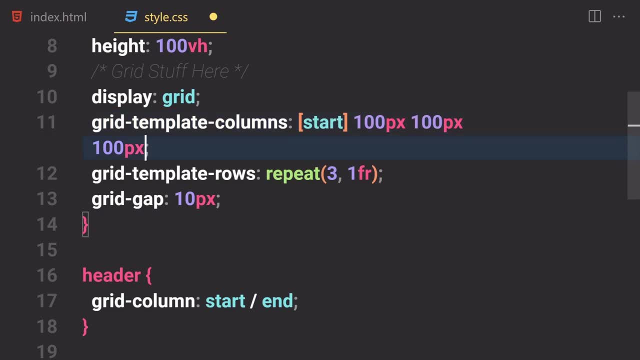 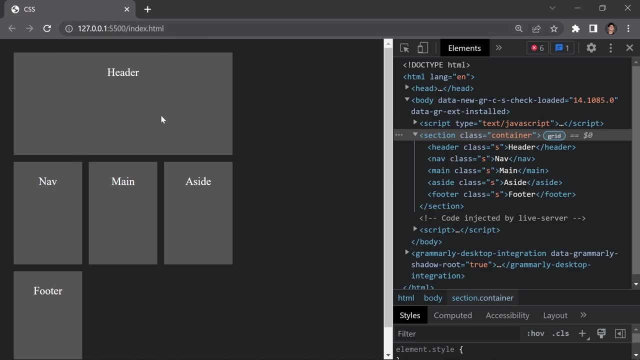 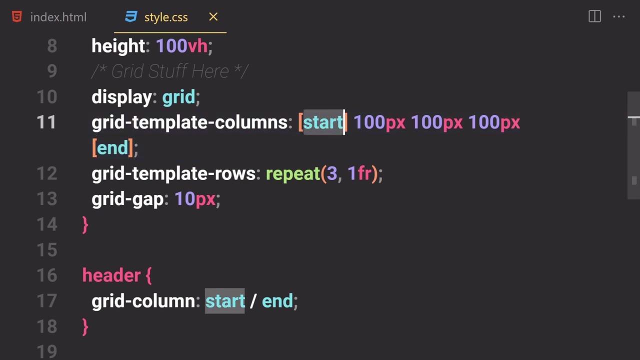 so for that we just have to cut this end name from there and we just have to put it right here, and if you save that and boom, it will now take up like three lines, like line one, line two, line three. okay, so you can play around with that if you want to, and you can also give him like any name you. 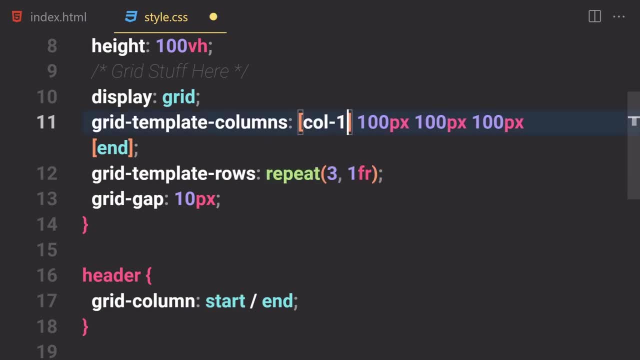 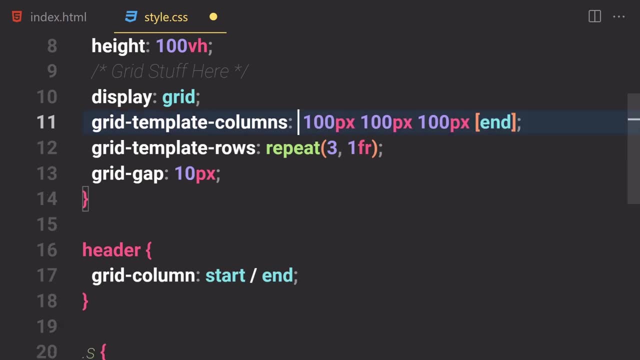 like: but in my case i just give him like starting and you can give him like call start one or stuff like that. but i just kind of want to show you like how you would name your lines by using css flexbox. so this is how we can name or line. so if you save that and we have to remove this property from, 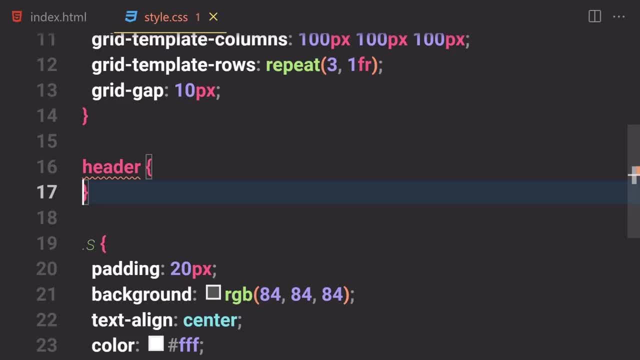 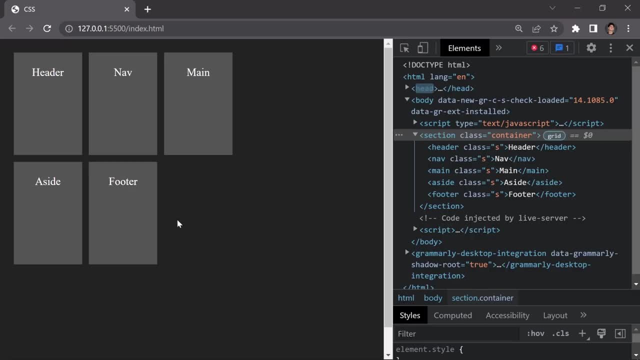 there, and this is how everything looks like now. and now let's learn about something called a min max function in grid. so you know what? first of all, let's just remove this header from there, and this is how currently things looks like, but i'm going to just set there to repeat function. 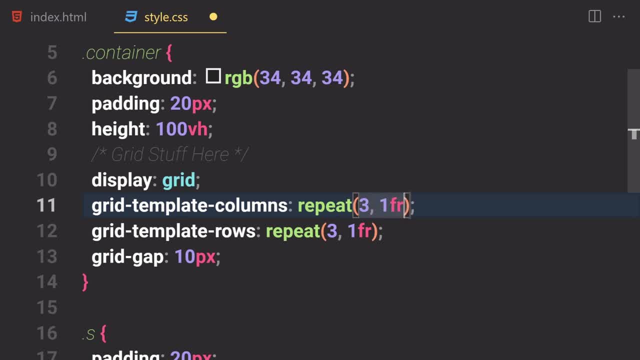 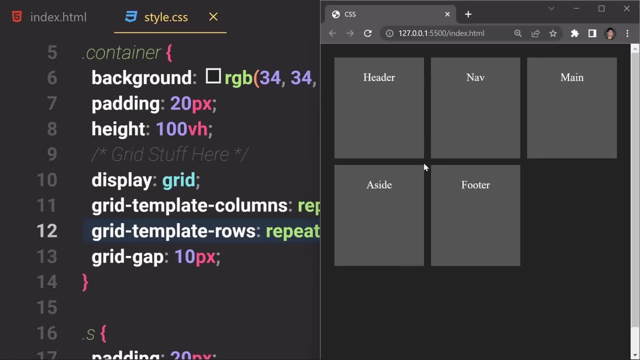 and i want to repeat like three times: and we want to provide one fr and rows are fine. so if you save there and now, if i just like make my screen size a bit smaller right here, so here you can see that items are also making smaller right here and we don't want that. in some cases we would want, or 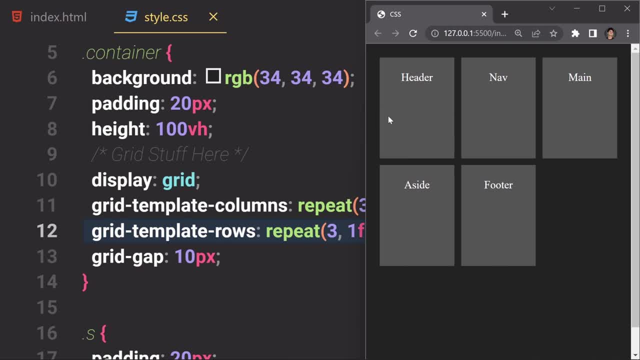 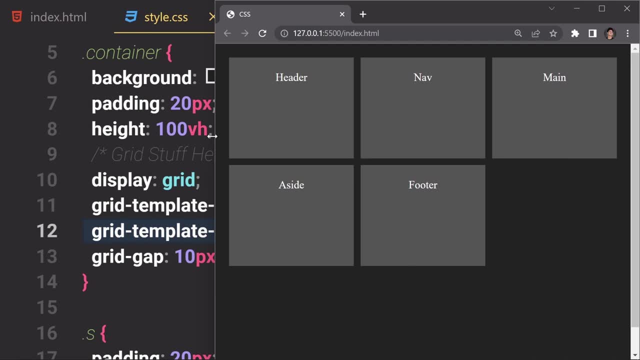 lines to be a little bit smaller, not alliance. why am i keep saying lines? in some cases we would want our elements to be smaller. in the majority of cases we are not going to be wanting like that kind of behavior, like if you just want to make your line smaller, you can make your line smaller. 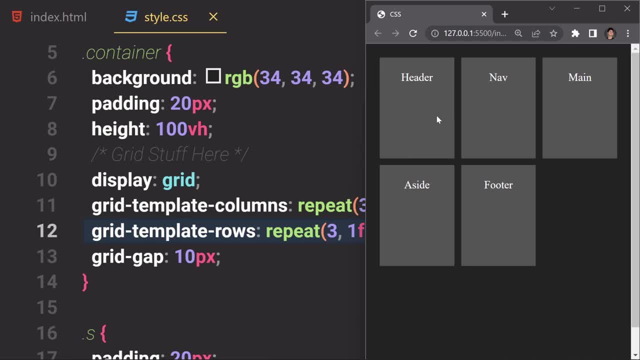 shrunk down or website right here. so here you can see, everything is now shrinking down as well. in a lot of cases, we don't want that same behavior, and so for this kind of situation we can use something called a min max uh function. so you know what uh? what do we have to do? uh? 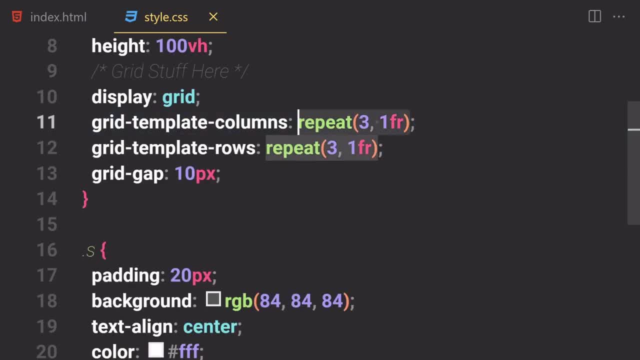 i don't know why did i write one far in here? uh, let's just try like um, maybe one fr, one fr and one afar, and if you sell that and i don't know what's going on, seven yep. my styling is back, so this is how currently things looks like. 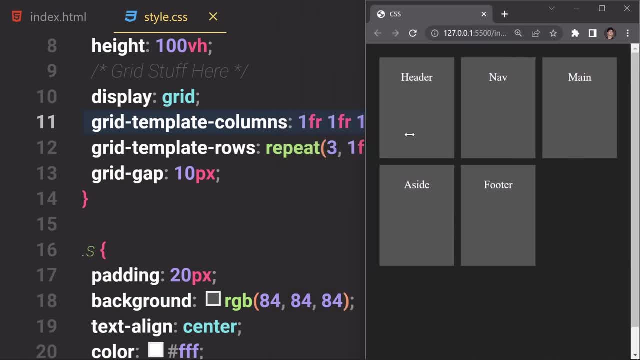 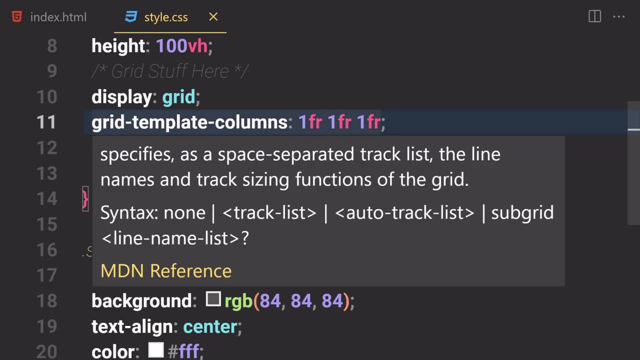 but if you want, like anytime we shrink or browser, and we don't want this one to shrink like this second element. so we want to provide a specific value for that. so for that we can just use instead of one ram, we can use something called a min and max function. so the first value, which 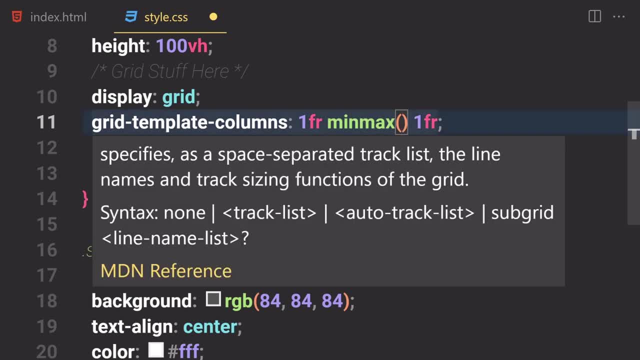 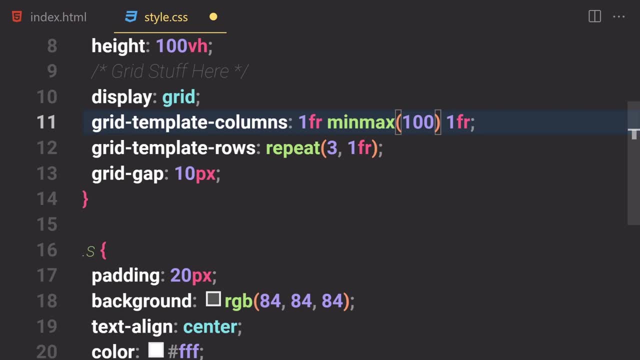 you are going to be providing for a min value and the next value which we are going to be providing is for the max one. so if you want to provide a value for the main one- so the main is height- will be like- uh, i don't know, 100 pixel will be just a little bit smaller. so i'm going to just 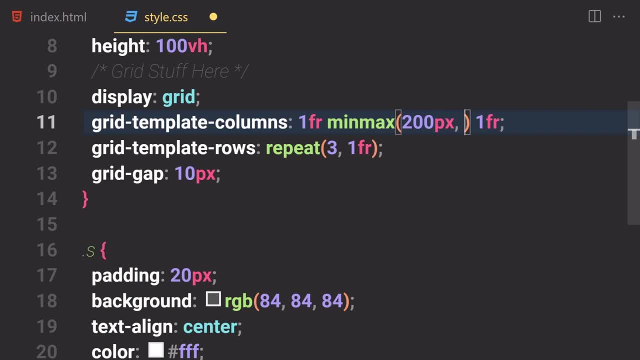 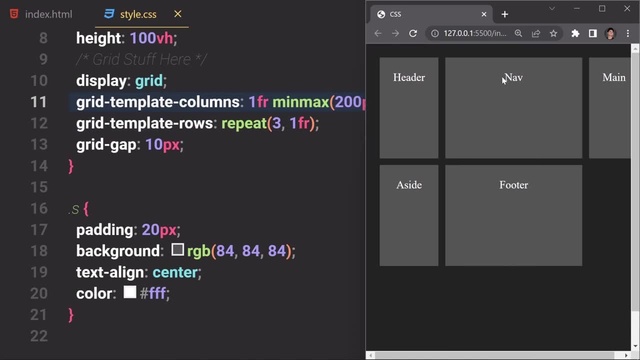 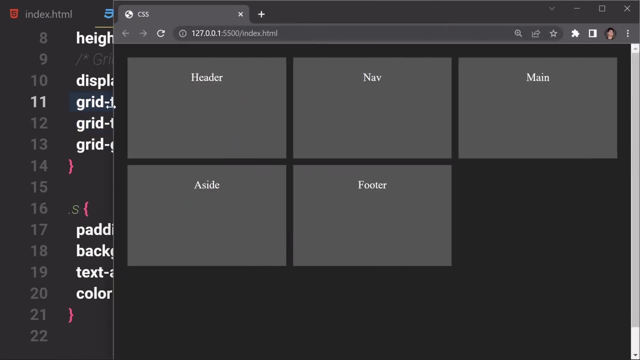 set that to like 200 pixel and the maximum value will be just one fr, like, however, the screen size is. so if you save that and here you can see, this one is now a little bit bigger because we specify 200 pixel width for that right here, and so if you just increase our screen size right here and it 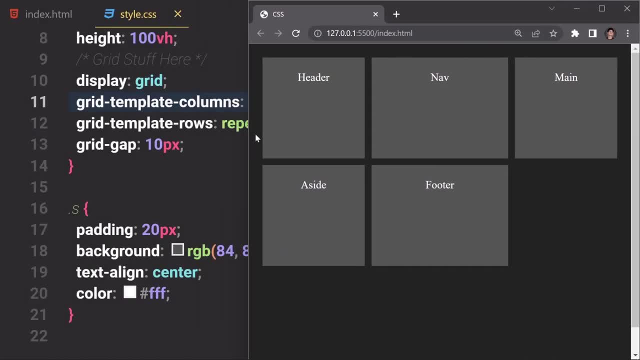 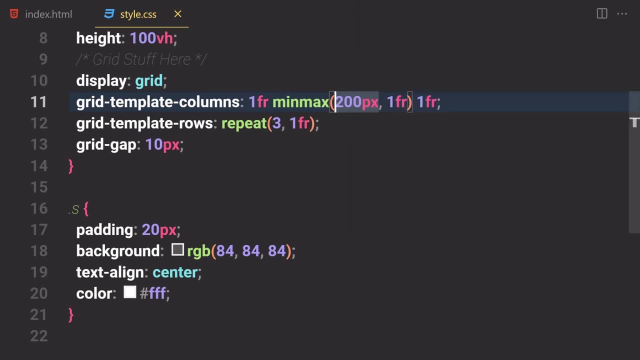 will now just, uh, grow up right here. okay, so if you just make it smaller, that other element will become smaller, but the middle one will not become smaller. that's because we provide a min max of 200 pixel for that. okay, so we first of all have to provide a minimum value and then we have to. 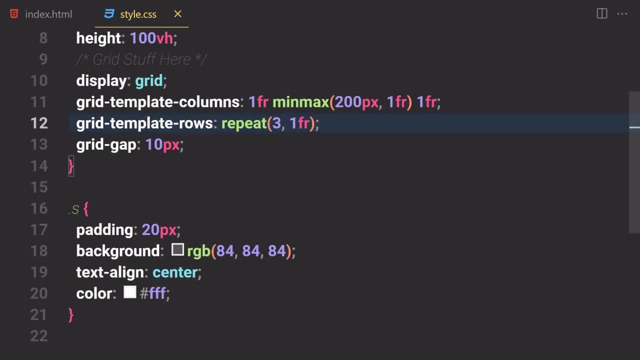 specify the maximum value. so this is how we can use a min max function, and this is a crazy function. you can use it all the time if you want to. so this is a min max function. now, the next property which you are going to be learning about is something called auto fill and auto fit. so, before getting 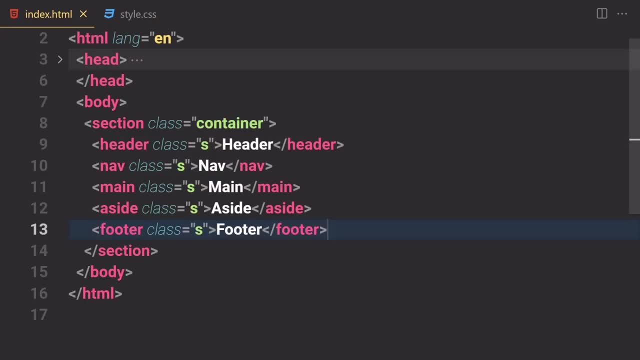 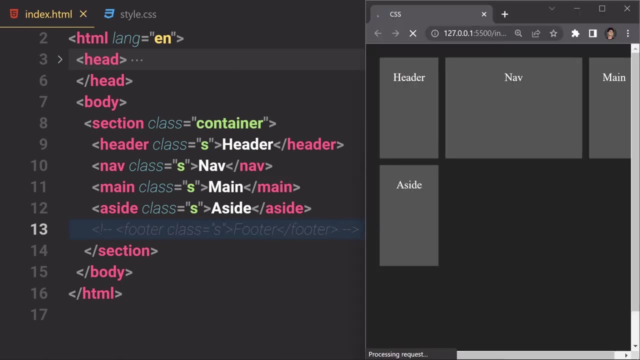 into the detail of that. first of all, let's just uh comment out a few things. so we have one, two, three and four. so you know i'm going to comment out this line and cell file and this is how currently everything look like and i'm going to 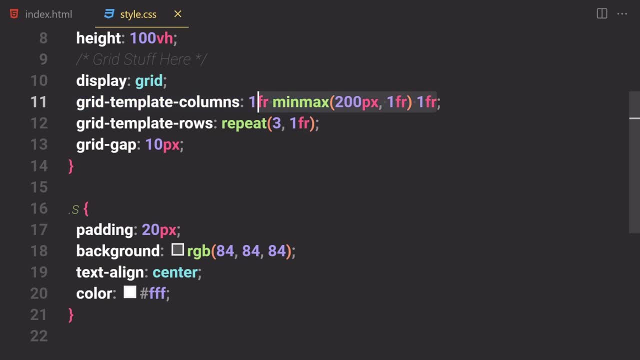 also remove that and instead of using like one of ours and one of ours, i'm going to put like 100 pixel right here, 100 pixel right there, 100 pixel right here as well, and i'm going to also put like 100 pixel right here, 100 pixel right here and 100 pixels. so if you sell that, i know we can. 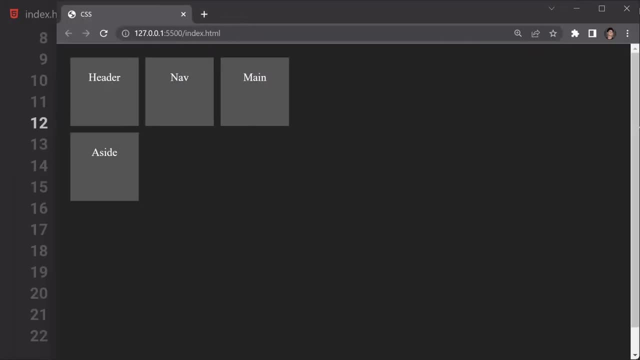 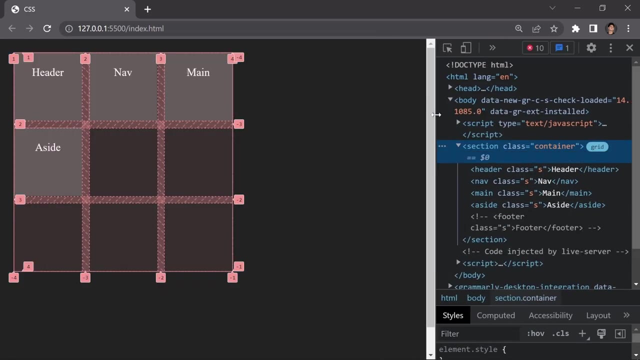 use a repeat function, but in this case we're not going to use a repeat function, so we're not going to be using a repeat function. i'm going to make it bigger. right click on it and then click on inspect, then select our grid area right here. so i want to show just the difference between us. 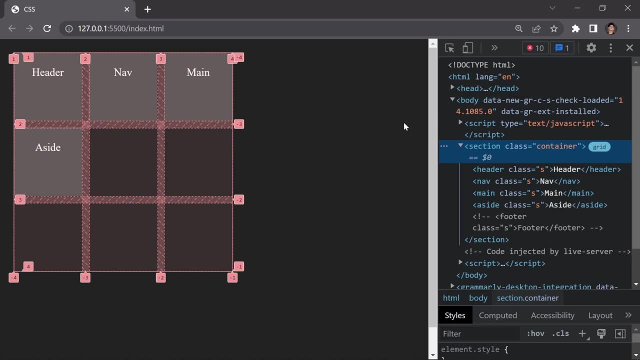 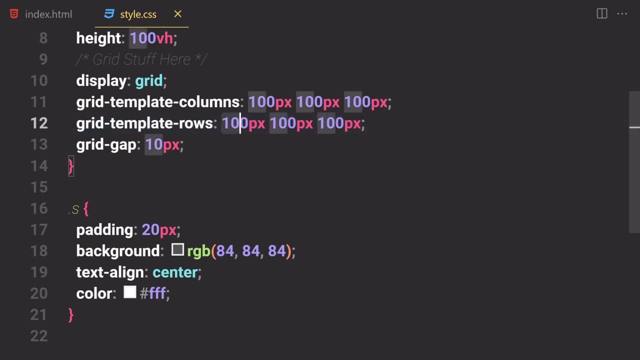 something called auto fit and out of fake. you don't have to worry about that much about auto fill and auto fit. but i just kind of want to show you what's the difference between all of the you know what? uh, let's just use something called a repeat function. for that we have to use a repeat. 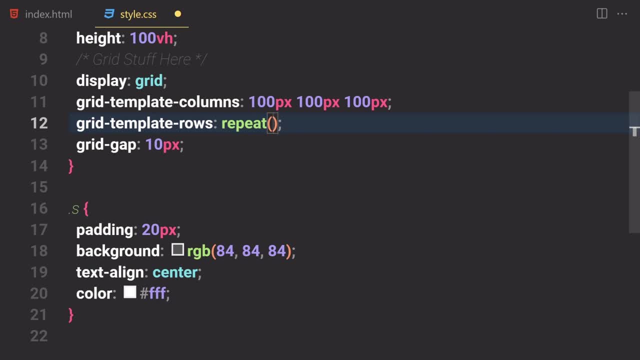 function. i apologize by just writing all of that code. so first of all in the repeat function we can just write like uh, auto and then fit. so if you just write auto, fit, and then we can specify like how much we want there, so we can just use like min max, or you know what? i'm not going to be using min max for now. 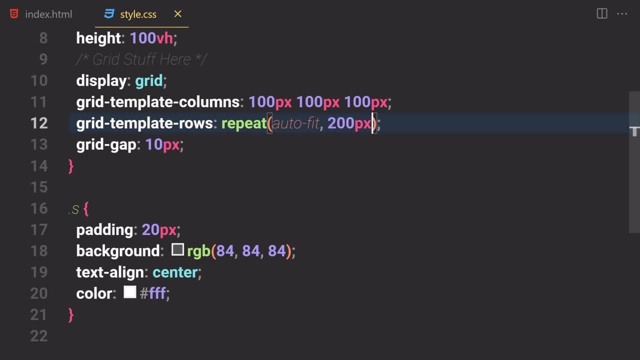 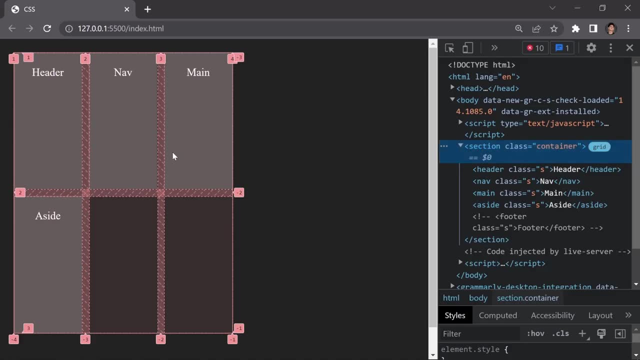 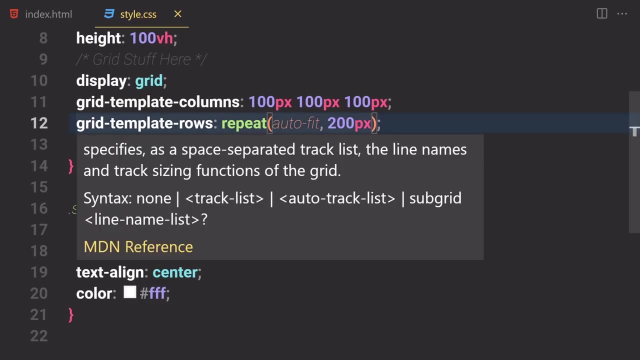 i'm going to just use like maybe 200 pixels, if you save that. and now, in this case, we are just telling our browser, like i don't know how many rows i want and how many columns i want, so i want you to just auto fit the content in this grid area. so for that we can use auto fit right here. 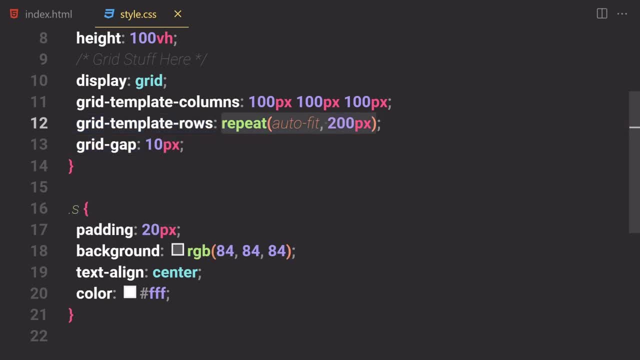 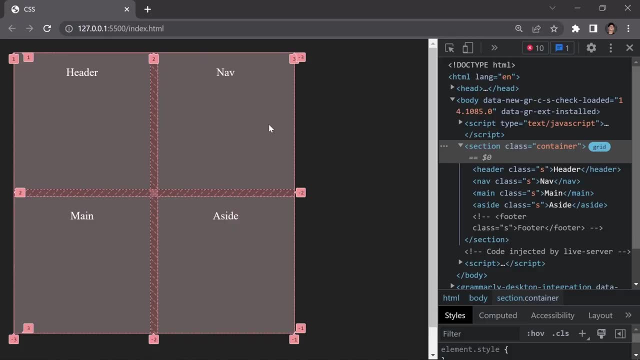 you know what? i'm going to use this function inside the column so that you guys can see everything a bit better and save our file. and this is how it looks like first of all. it will now just give us two rows right here, so if you want to shrink there to like 100 pixels, save that. 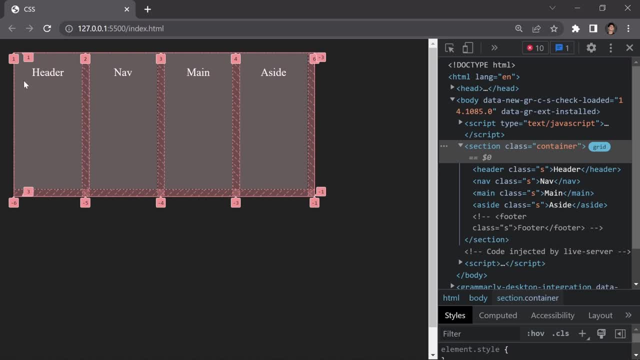 and now, here you can see, it will now give us, uh, what do we call it? uh, four rows right here and two columns, and it's not shrinking down, i don't know why. so if we just provide a hundred pixel height to it, uh, you know what i'm going to comment this like? oh no, we're not going to comment it out. 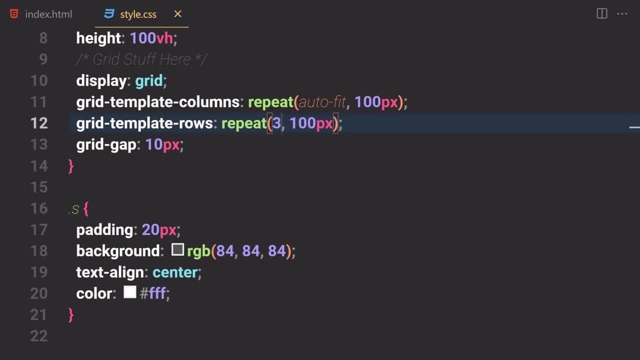 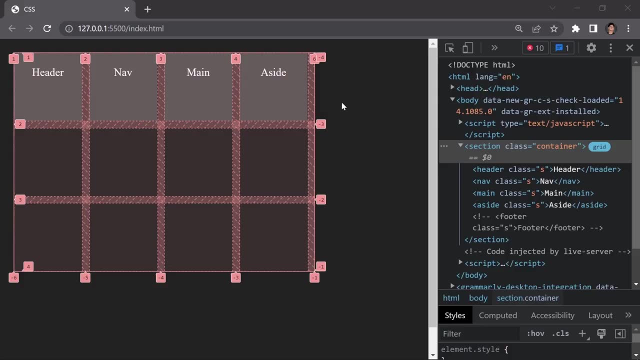 so i'm going to comment it out, so i'm going to comment it out. so i'm going to comment it out, to just put that like, maybe three in there. and if you save that certain log uses three columns and four rows right here, that's because of that. auto fill, uh, auto fit content property right here. 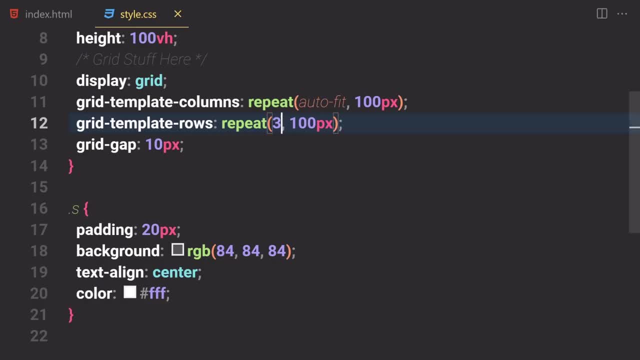 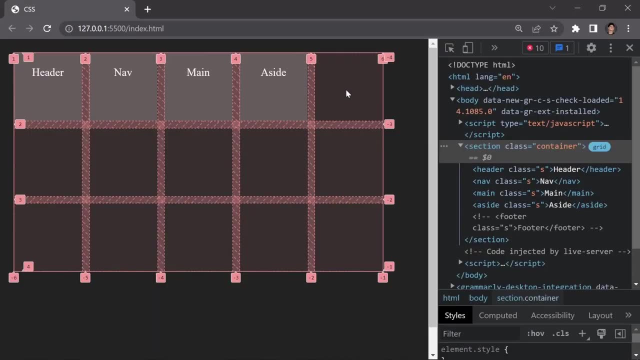 and here you can see. we don't have any other uh kind of boxes right here. but instead of using auto fit, if you just uh select like auto fill and if you save that, so here you can see, the log uses another uh element right here. so if you want this second one, like this one, to go in here so you can. 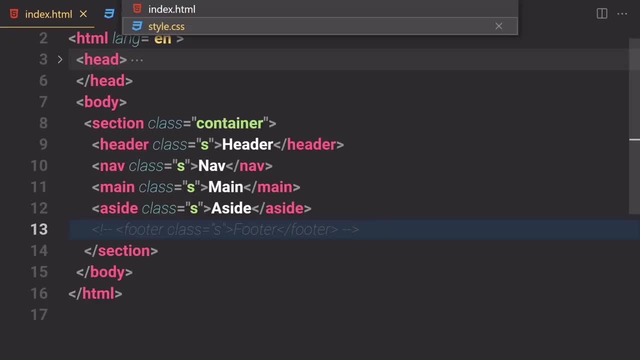 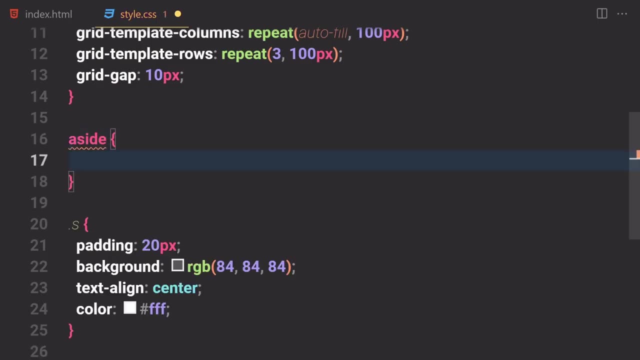 also use that. first of all, let's just select or aside, so we have to just use. i guess the final one is aside. yeah, it is aside, so we can just use a side. and here we can just provide a property column, and here we just have to write like a grid column, and then and, and here we just have to. 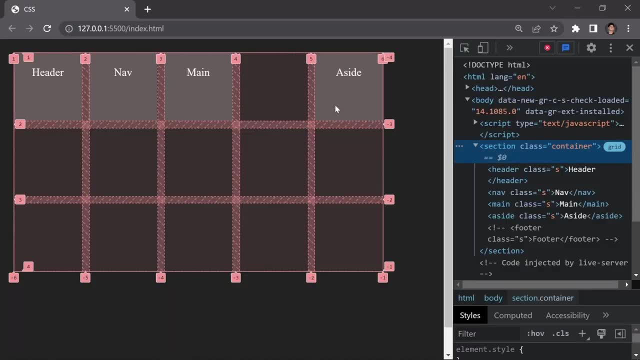 specify minus two and if you save that and we'll push this item right here and now. if you just change this property instead of auto fit- i mean like auto fill- and if you change that to auto fit and if you save that and here you can see, it will now remove that right here and you can just 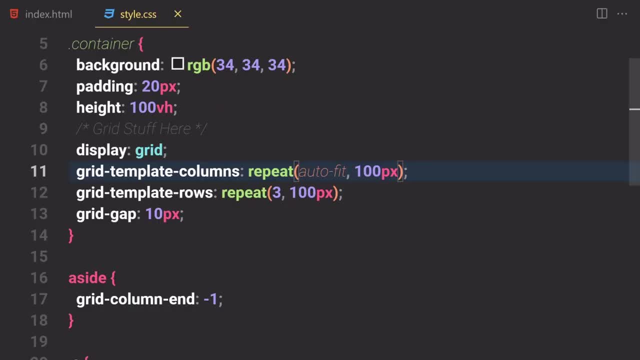 from here so we can increase and decrease the sizes of order element, and it will just. our browser will by default figure out like how much rows and how much columns do we need by using this auto fit and auto fill property. and i know it can be a little bit confusing at first, but you. 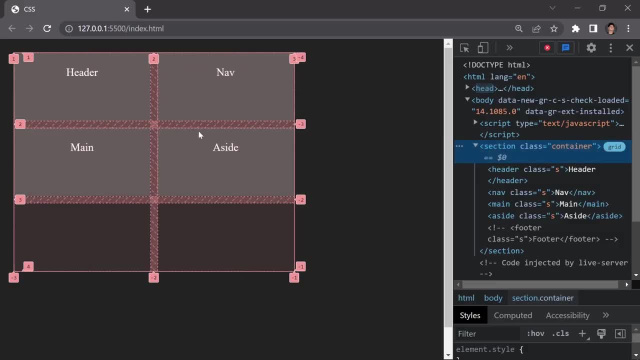 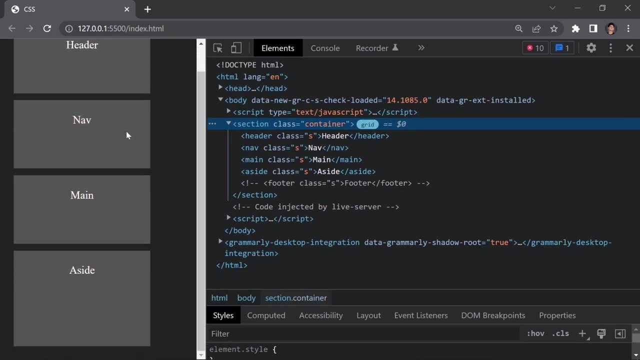 don't have to worry about it for like that much. so if you save that, so here you can see, browser will figure out everything by itself. so if you just shrunk down or screen size right here, so our item will also shrunk down as well. okay, so this is how we can use auto fit and auto fill. 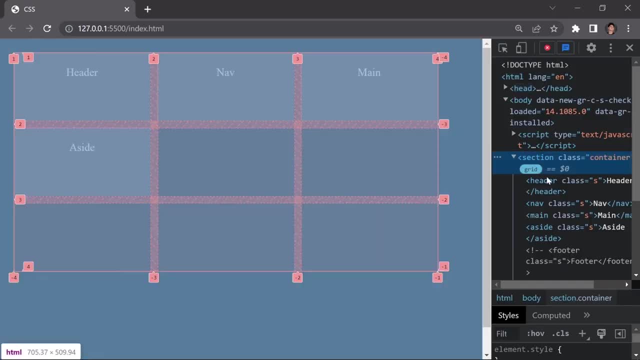 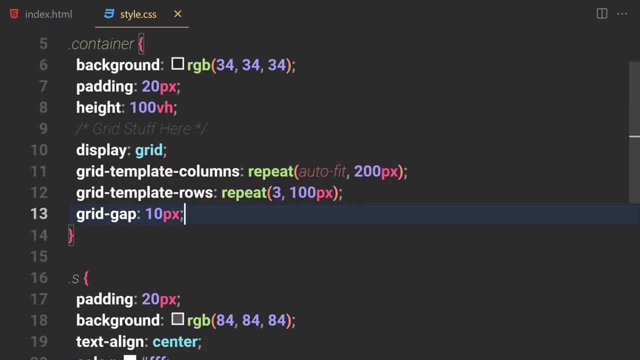 and i'm going to remove this aside from there and boom, all right. so now the next thing which you are going to be learning about is something called a flexbox thing. so now that we know enough about a css grid for now, so we can also use a css flexbox property, which we learned just a second. 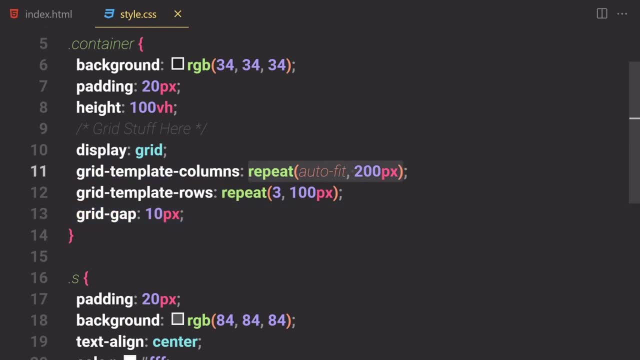 ago in our css grid, if you want to. so that's why a grid can be a little bit powerful than our css flexbox, so we can just write a you repeat in here and we just have to write like maybe three rows. i'm going to just set that to. 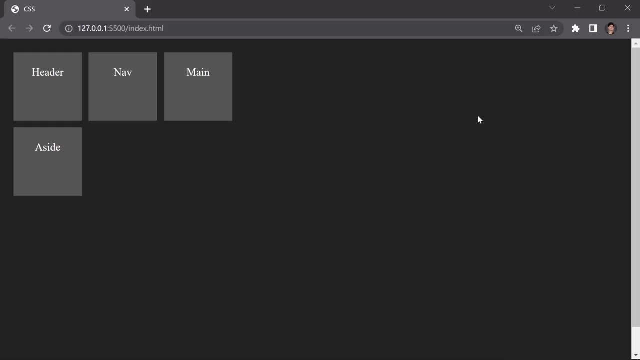 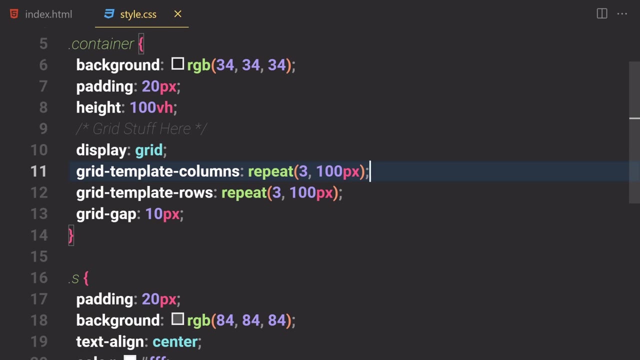 like three and comma hundred pixel would be fine. so there, and we can use that justify content and all of their properties, which we learned just a second ago in a flexbox section, so we can also use it right here if you want to. so you know what i'm going to. just start from the first property. 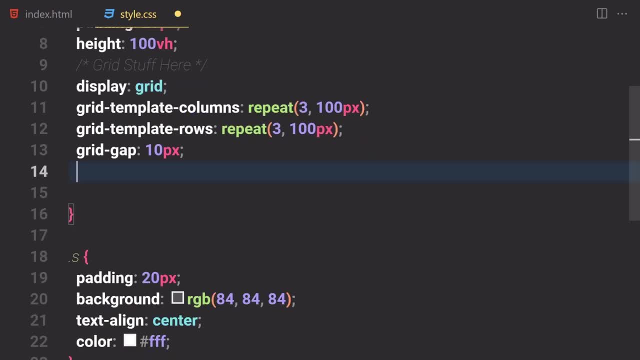 which is known as a justify content, and you already know, like, what a justify content property will do for us. so we just have to write like a justify content in here and we're going to use that as a justify content and we can have like our center end and start, like flex start and flex end. 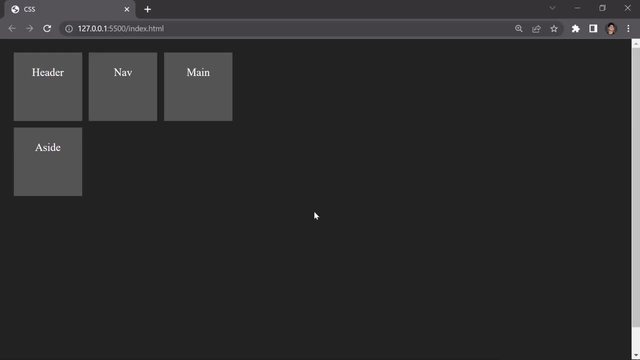 if you just write like a flex start and if you sell file, this is the default one. if you just set that to flex end and if you save there, so it will just push it to the end. we can also push it to the center if you want to and stuff like that, and we can also write like a space uh around and if you. 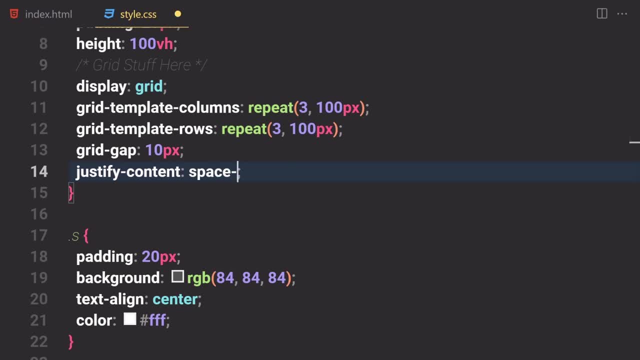 save there, it will give us a space around in each item, or in each cell to be precise, and if you just write like a space between, save it, so it will also give us that spacing between the two and then we'll have like a space between that justify content. so this is it about justify content. you already know. 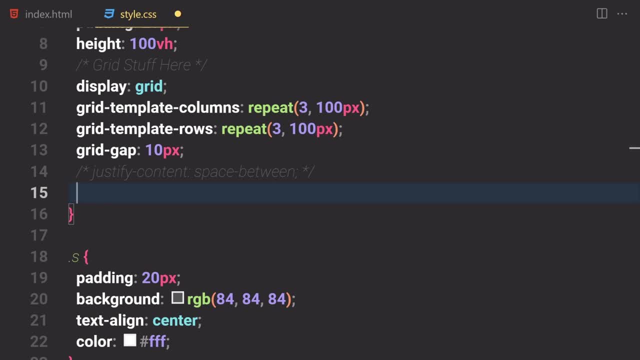 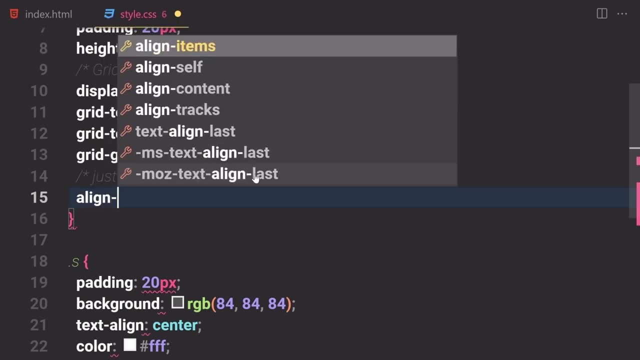 that i don't want to waste your time one more time. so if you don't know that, you can either just click google search or you can just watch the flexbox section if you want to. and so now let's just learn about align items properties so you can also use that aligned items property in a css. 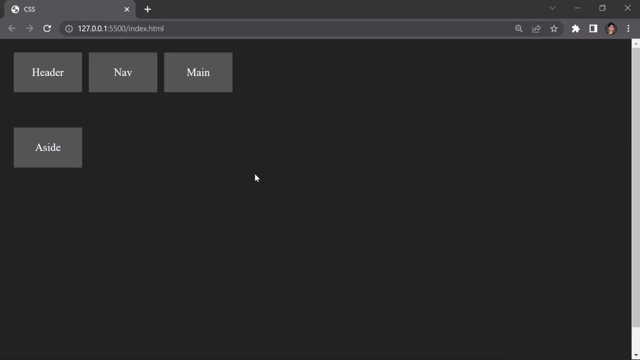 grid as well. so we have, like flex start and if you saw that- and this is going to be the flex start, we have a flex end and it will now push it to the end. we can also have a flex center right here. so here align item center, so it will now make it center and this one will be just- uh, let me just 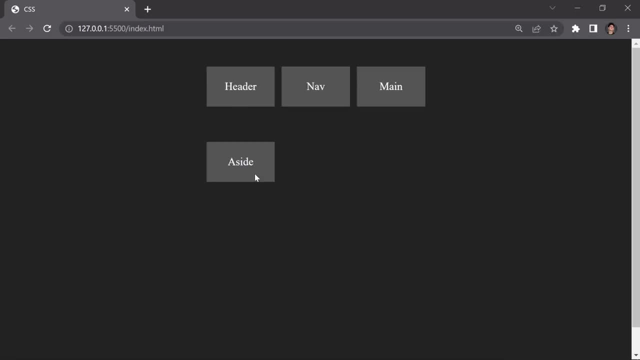 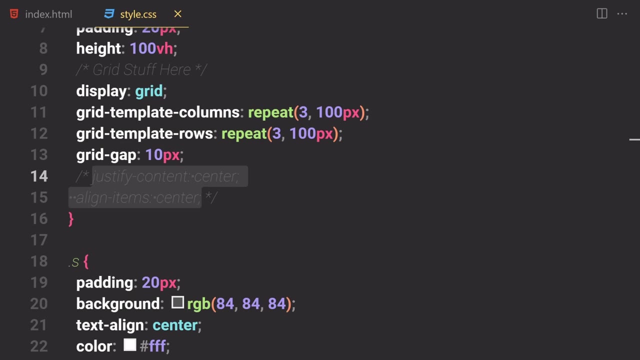 write a centered center so you guys can see everything about clear and here you can see it will now just make it perfectly centered. so this is it about for justify content property and align items property, and we also have that order and align items and justify item and stuff. 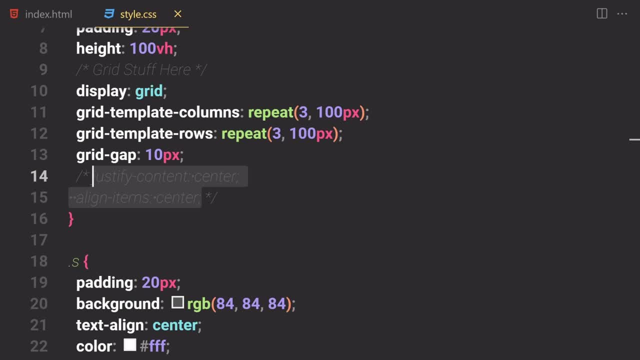 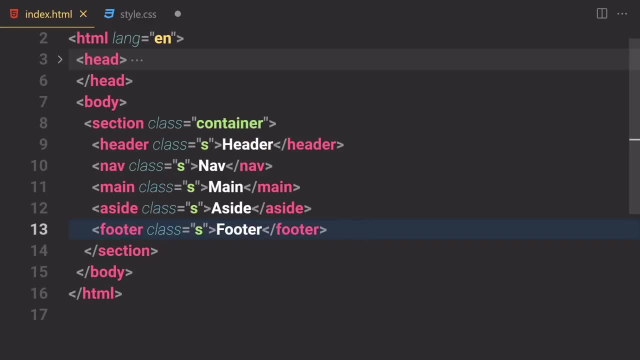 like that, like align self property and all of that stuff which we already learned. so now let's just use that order properties, so let's just select, or uh, so you know i'm going to use the order property and i'm going to provide this photo right there and let's just select this aside one. 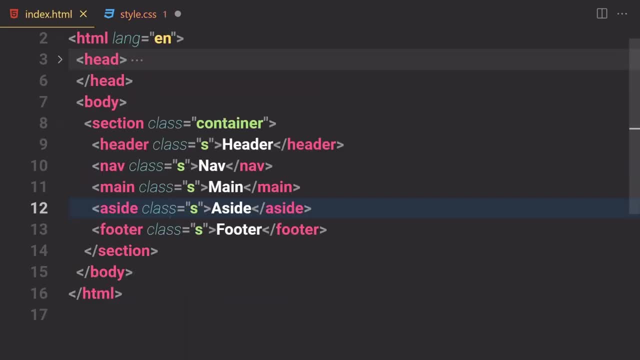 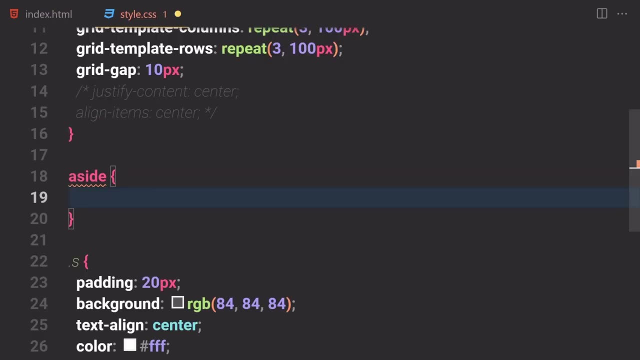 right here, so i'm going to just select my aside. we already know that if you use like display of flags or display grid, so all of them will have the order property by default set to zero. so we can also just increase or decrease that if you want to. so if you want to just write like order, 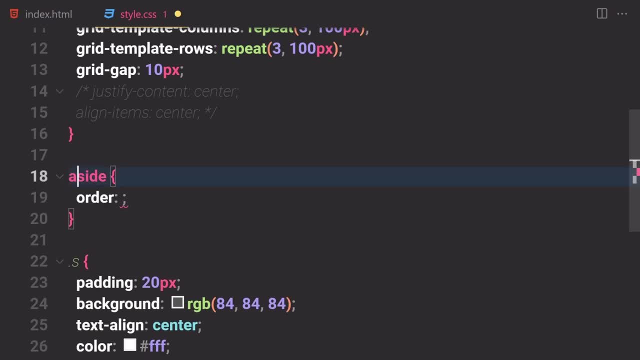 and here you can see our aside is now right here. or you know what i'm going to? just select my header so you guys can see the difference between all of that. and here you can see, header is now at the end. we can also push it to the bottoms by just providing one to it and boom, here you can see our. 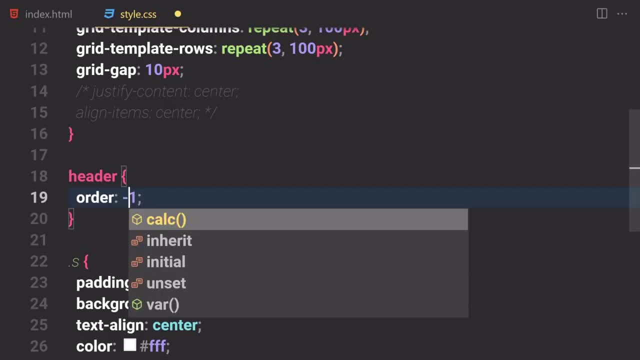 header is now at the end. we can also provide negative values. so if you save that, it will push it to the top as well and we can just provide. like you know, i'm going to remove this minus sign from there and now let's just select, maybe, this main area. so if you just select our main and if 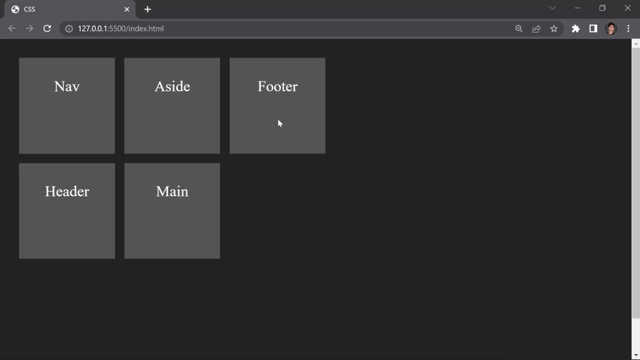 you just provide an order property for that, like two, and if we save that, and it will now push this main to the bottom right here, because this one have now the highest value, like this, one has two, one have one and these, all of them, like these above one have, uh, zero. so that's how we can play. 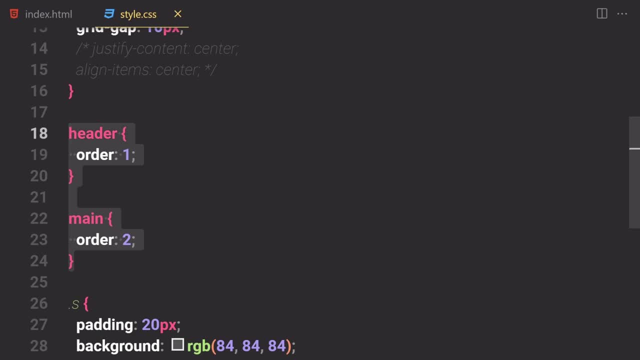 around with the order property. so now the next property which we are going to be learning about is something called align self property and we already know, like what align self will do for us. so i'm going to comment this main for now and we can just use like align self, and here we can just 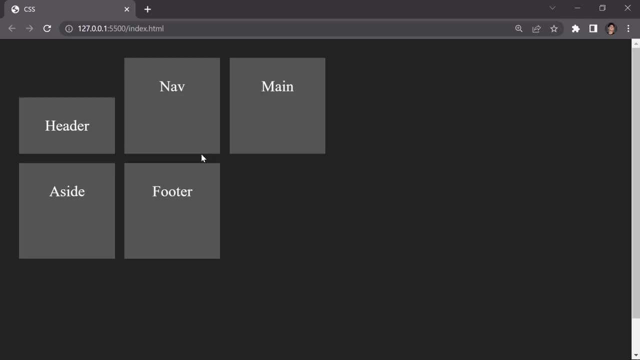 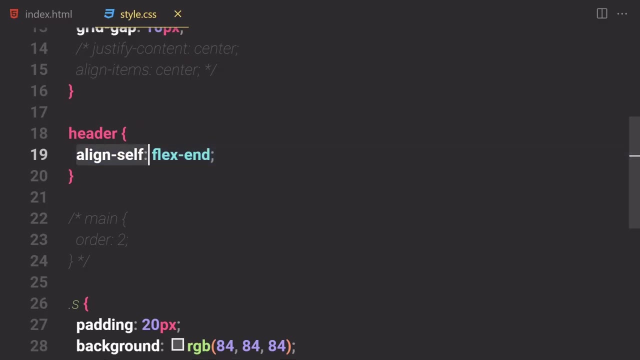 write like: uh, maybe a flex end, and if you save that, so it will now push its item like that one item, like one single item, because in this case we are working on align self and it will just work on a single element inside that container. so we 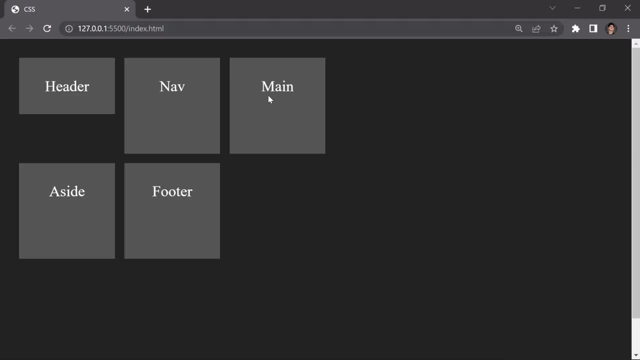 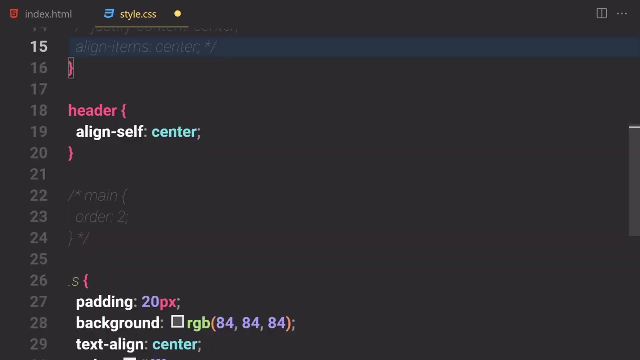 can just write a flex, and we can also write a flex start and we can also write a center if we wanted to. so center and if we save that, and we'll now push this item to the center. okay, so we can also use a justify itself if you want to, but i'm not going to go into that much detail. all right, so 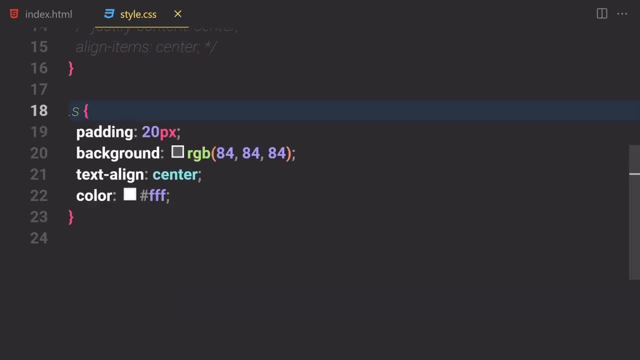 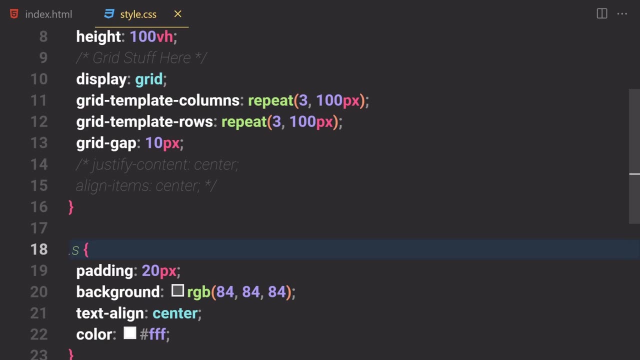 now that we know enough about css grid. so now the final property which we are going to be learning is something called a css grid and css grid is something called a css grid and css grid is a css grid. uh, not a css grid, but css template areas property. so i'm going to just remove that from. 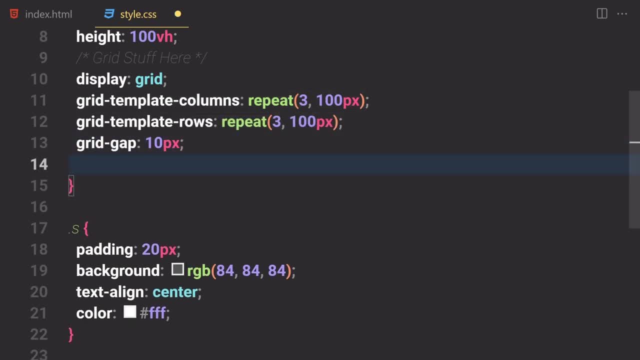 here and we are going to start working on a css template area property for now. so now let's just learn about something called css template area property and, as by now you already know, like what is a template area or css grid area? we already learned that in the slide once we were starting. 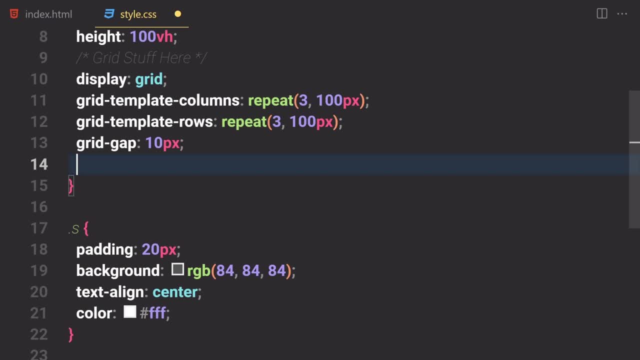 this tutorial. so the grid template area property specify area within the grid layout. so if you want to create a grid layout, you can create a grid layout. so for that we can just use or grid template. let me just write template and then areas right here, and this is just a little bit weird. you have 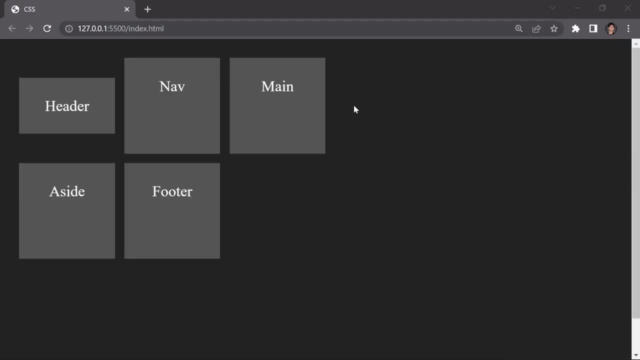 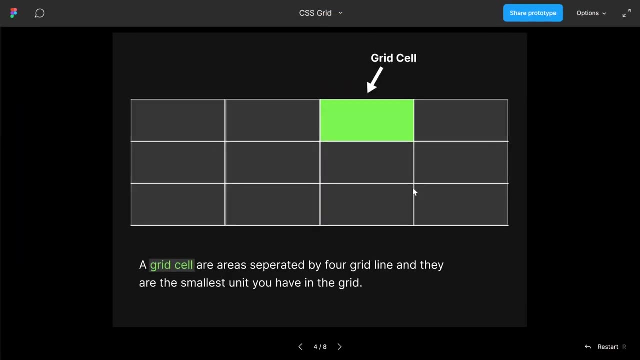 to keep that in mind. so this is just a little bit weird. so before getting into a lot of great details, first of all let's just learn about, uh, let's just discuss, like, what are we going to be building in this kind of a section? so first of all, let's suppose: if you want to build this layout, right? 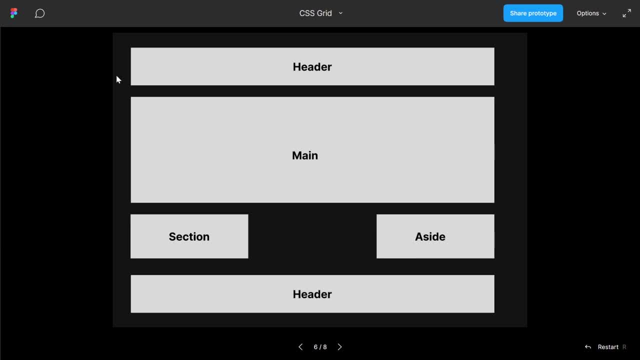 here. so how can you go about doing that? so here you can see, this one is taking its place. this one is also taking like two rows right here and this one have one uh item in here. we don't have any item inside at the middle right here. 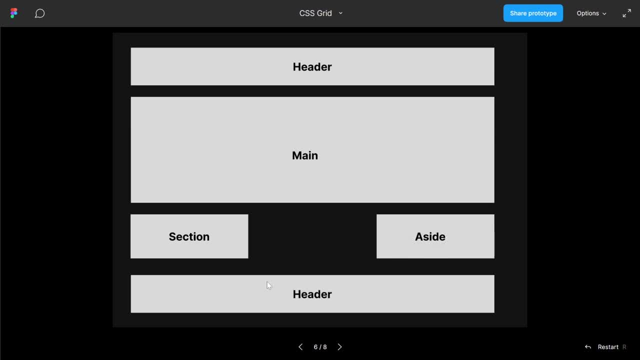 and we have one item at the end and finally this- uh, i write it ahead- and finally, this footer area is also taking its place right here. so if you want to create this kind of template or this kind of layout, so for that we can use a grid, template areas, and it allows us to provide an area for us. 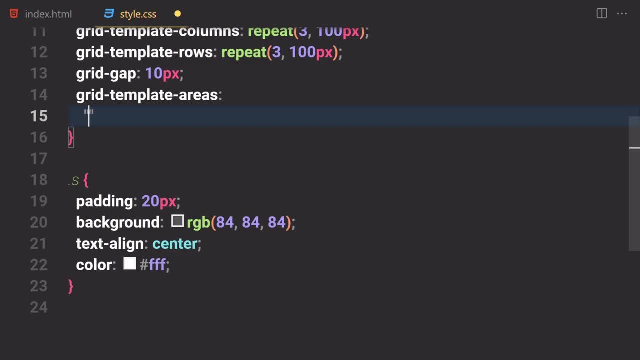 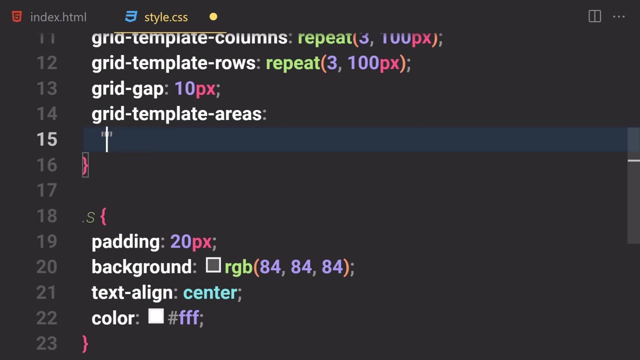 okay, so first of all, let's just use: uh like, let's suppose we have a header, so we are going to be specifying: header, header, header. you can also go with a header if you want. you can give any name you like, it doesn't matter, but you have to put something in here. so in this case, instead of writing totally a header. 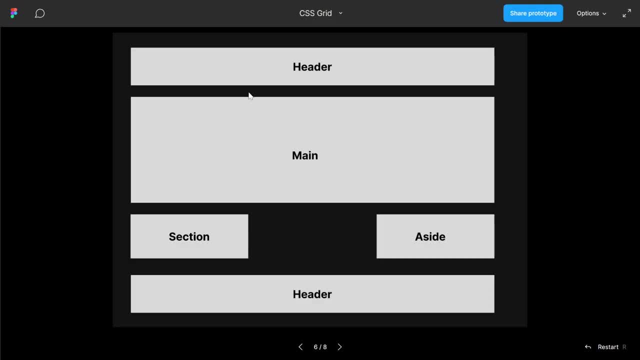 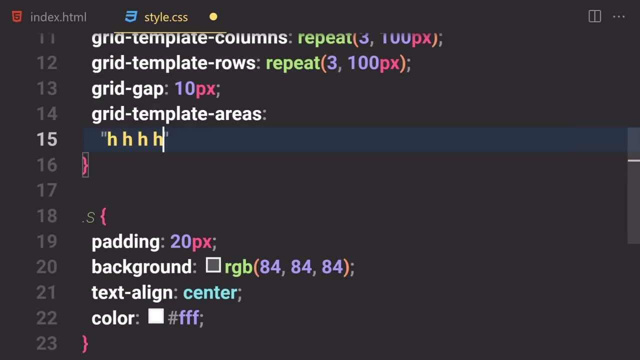 so i'm going to just write h, h and h. so what does that mean? h will start from the first line, it will take a second line, then the third line, and we can also just write like fourth line. and, by the way, if you're working on a grid- template areas- you have to remember your row. 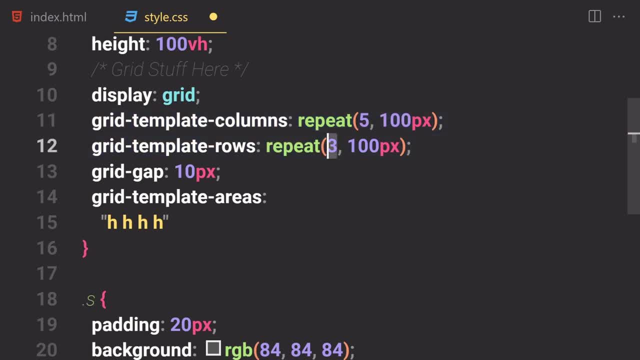 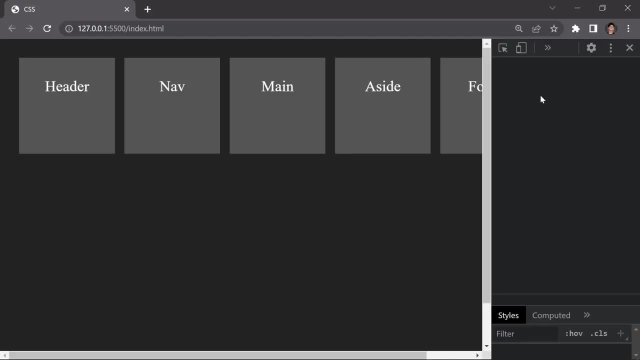 and columns. so in this case i'm going to set there to like five and five and, by the way, i'm going to comment this line out for now. and if you save that, and now let's just check out our browser. okay, so if you just click on this grid right here, so here you can see we are now getting. 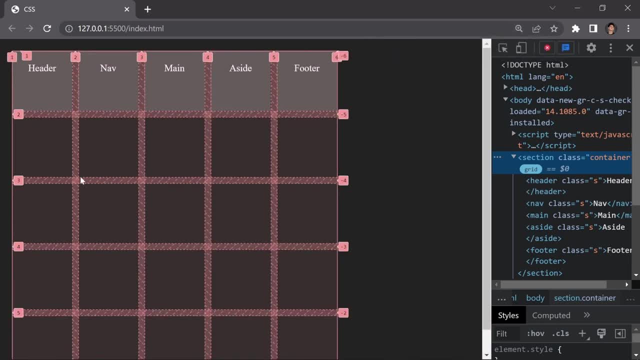 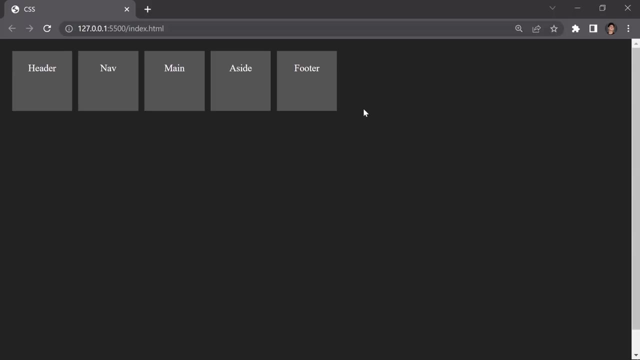 um, five rows, uh, five rows and five columns as well. okay, so this is it. you know, i'm going to change this one to: yeah, i guess five would be fine. so now that we specify that, now let's just use this h in or header area, so if you just save this property right here. so here you can see. 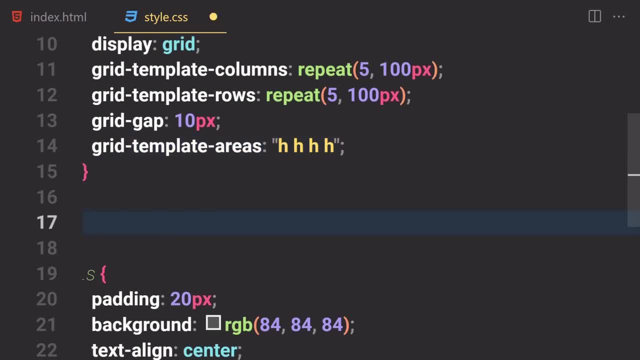 we still nothing is happening, and so if you want to work with a grid template area property, so for that we have to learn about another property called just a grid area, not a grid template area, but just a simple grid area. okay, so let's just select our element, like maybe header. 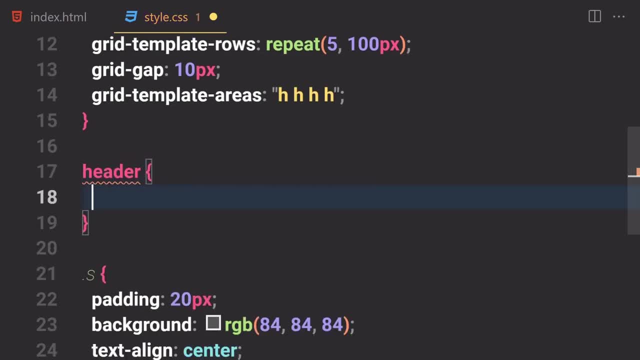 would be fine. so if you just select our header right here and we have to just use our grid area right here- not a grid template area, but just a simple grid area. and what is this grid area? so the grid area property specifies a grid item size and 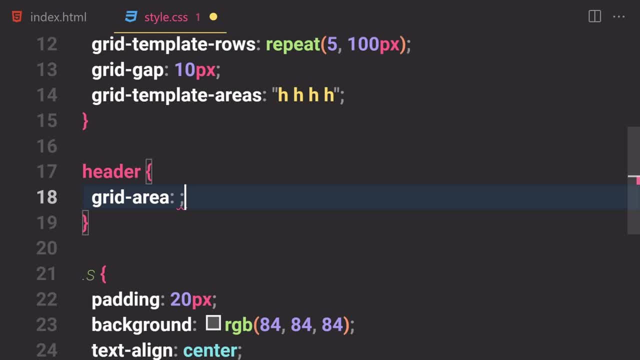 the location in a grid layout and this is a shorthand for writing a grid row start, grid column start and then a grid row end and grid column end. okay, so this is a short hand for all of that. so instead of writing on that header and stuff, so we can just provide h right here. 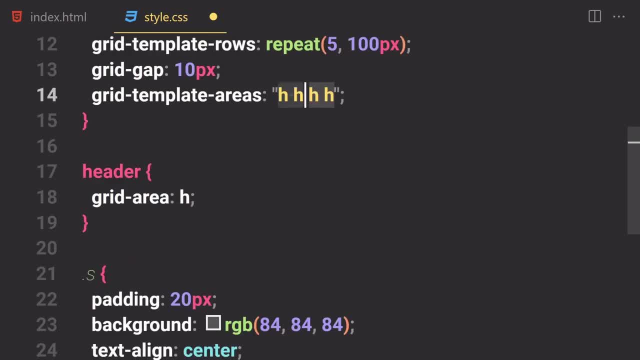 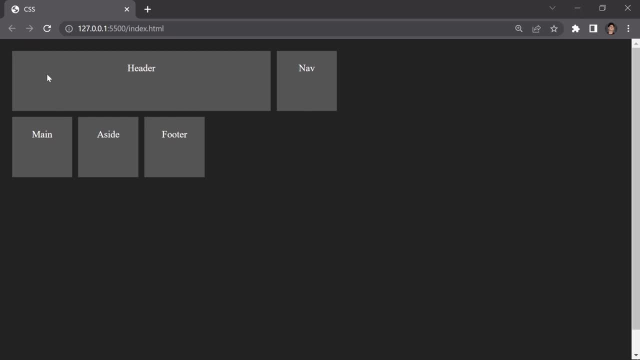 why? because we provide this edge right here, we declare that right here and that's why we are using it right here. and if you save that, and here you can see, it will now take up these lines. so why, so why are you taking all of their lines, if you just right? 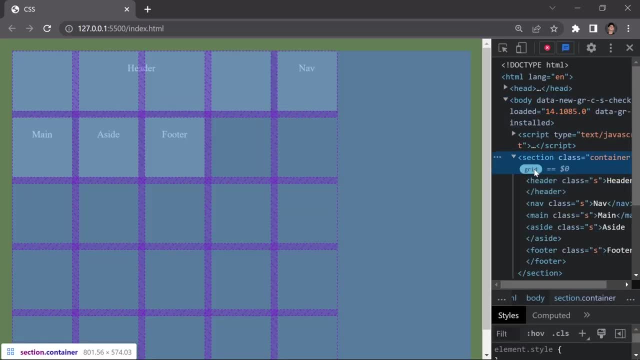 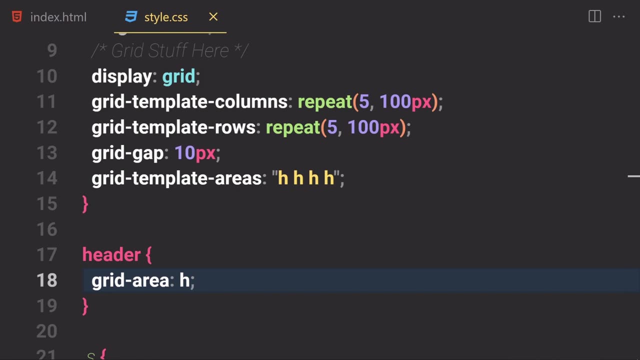 click on it and go to inspect one more time and if you just open your grid area right here, so it's now taking like line one, line two, line three and also line four right here. why is that? because we use this h four times right here. so we have line one, line two, line three and line four. okay, so if 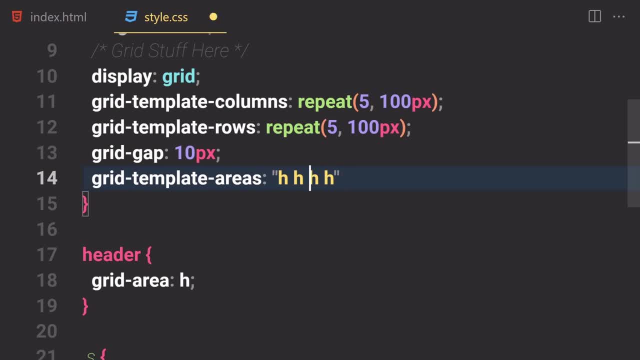 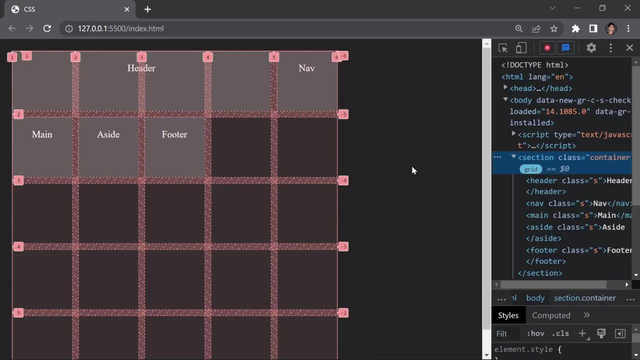 you want that other items to also take its place, so for that we can also just use that for for that. okay, so i'm going to just hit tab in there and if you just write like: maybe i don't know if you want to grab this one like main area, so for that we can also use first of all h, h and also. 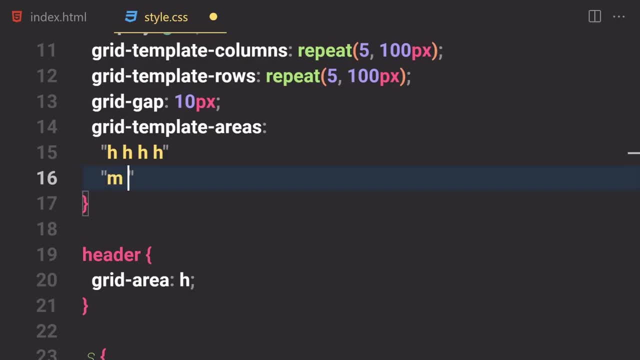 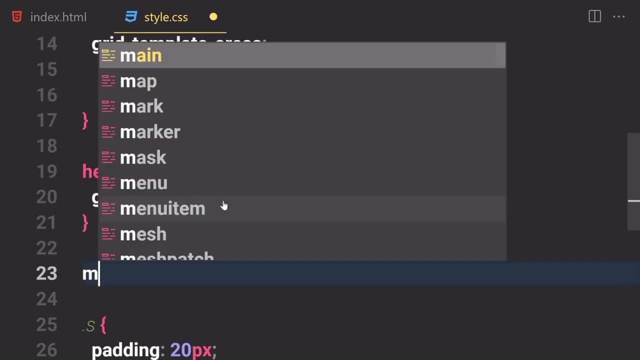 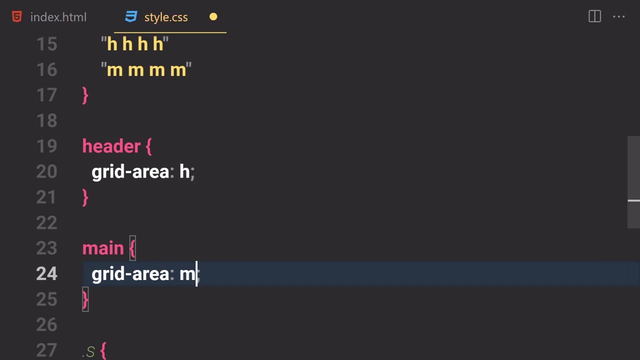 not h, but it's a main area. so there we can use m, m, m and m, so four time m, and now we just have to select that main area. so if you just select our main area, 00000, настолько, now let's just select our grid area property right here, and here we just have to specify this m, right? 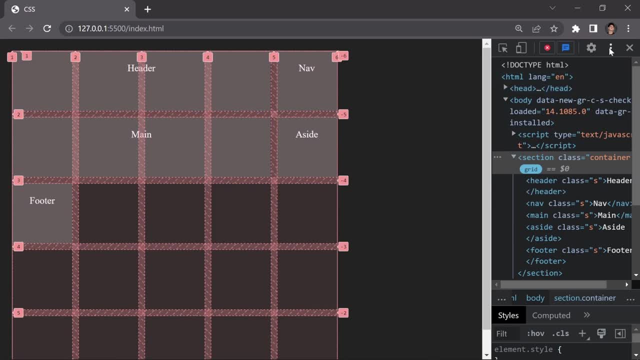 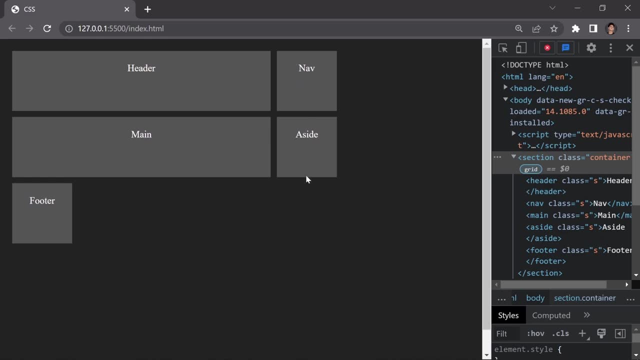 here, and if we just save that? and now let's just check it out, and here you can see this m is already taking this area right here as well, but here you can see, we have these elements right here stuck in there, so for that we can just remove. uh, you know, i'm going to provide a four column layout. 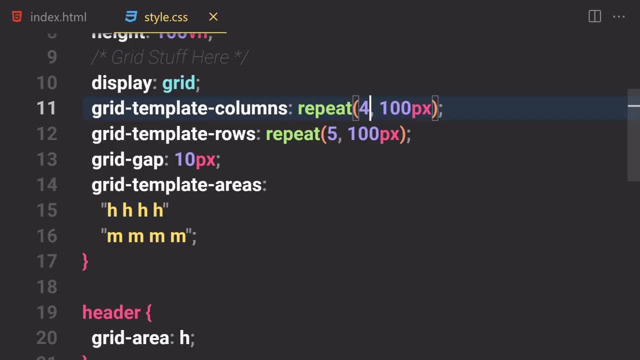 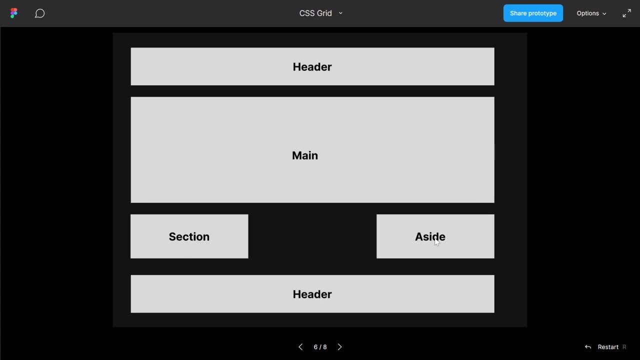 and we'll now push it right here. okay, this is kind of it, but now let's just work on a period one. so we have our section right here and then we have nothing inside there and then we have our aside. so if you want to go with this layout, so for that what do we have to do? we have to just write our. 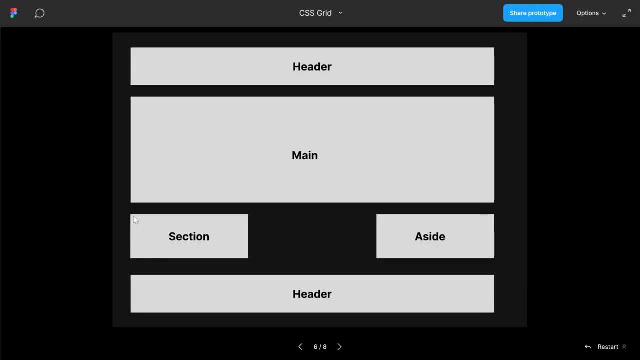 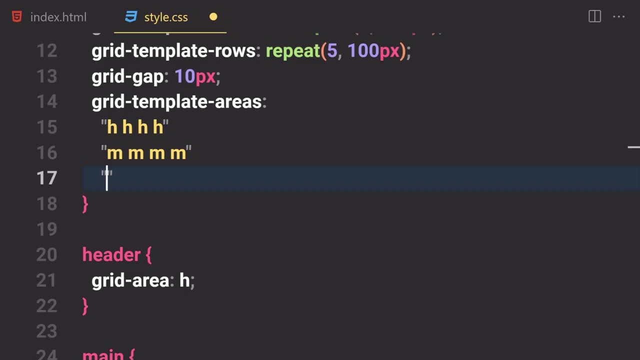 new string. so what do we have? first of all, we have section taken its place from one line to maybe two or three line, and then we have nothing, and then we have our aside from one and two. so now let's just use that. so we have first of all our h, then not h. it's a section. so we just have to write s. and s. and if you don't want any content whatsoever, you can just write s and s. and if you don't want any content whatsoever, you can just write s and s. and if you don't want any content whatsoever, you can just write s and s. and if you don't want any content whatsoever. 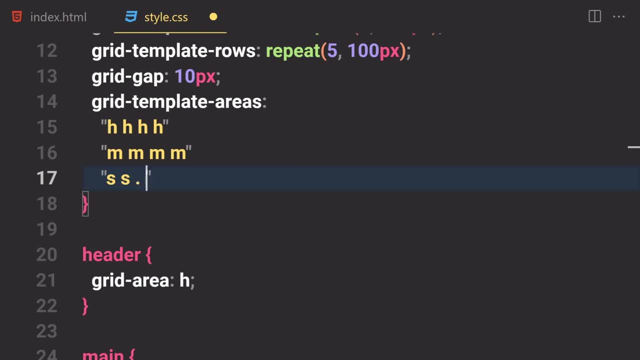 inside some sort of a cell, so for that, we can just put a period right there, or dot, whatever you want to call it. and now what do we have to do? we have to select this aside area, so we have to just write a right here. okay, so now we have to use this s and that a, so for that we are going to be. 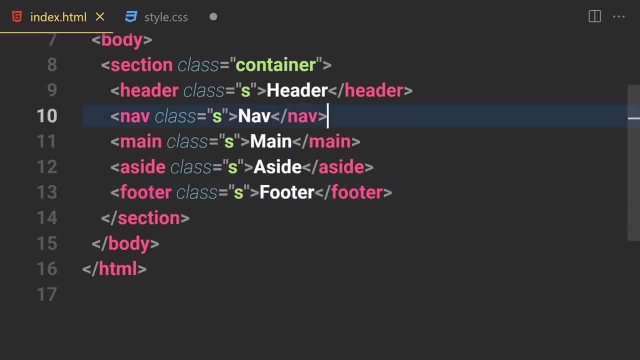 selecting our uh section. okay, so we don't have any section. you know what? i'm going to remove this uh nav from there and i'm going to put that a section and i'm going to just write like a section inside there and i'm going to put it right here at seven. here we have to spell. 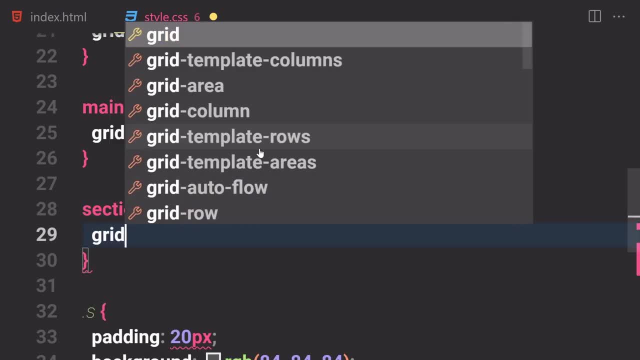 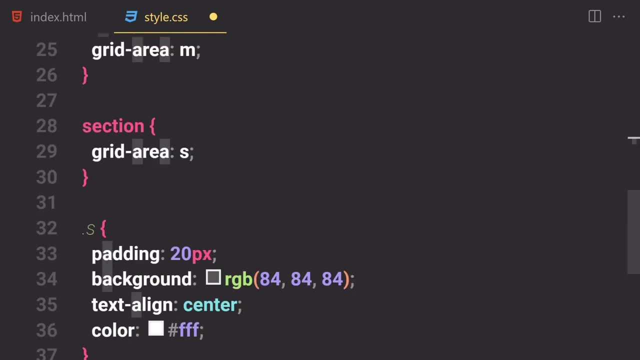 that section. so we are going to be writing a section and grid area, and now let's just put our s in here. and what else do we have to do? we have to select our anchor not anchor but or aside and we have to specify the grid area property for this. we are going to be selecting or assigned, and now 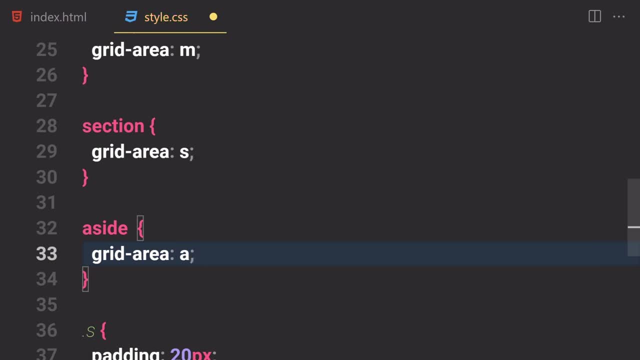 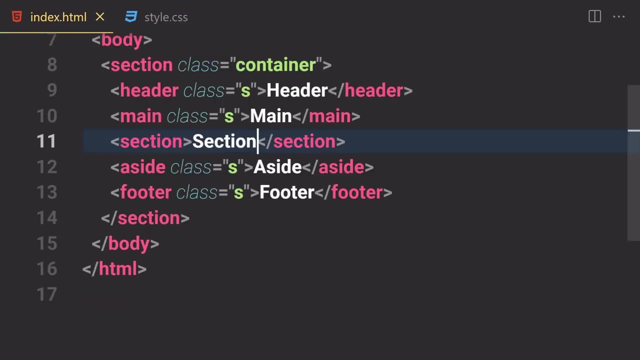 let's just use a grid area property of the inside, that aside. so we just provide that a for that, and if you save that- and here you can see, i guess something went wrong, because we didn't provide any style for that. so now let's just use class. 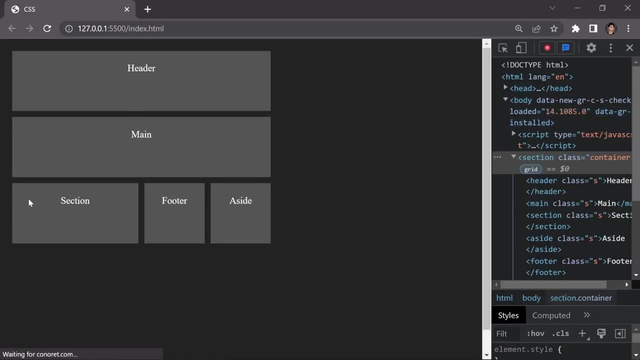 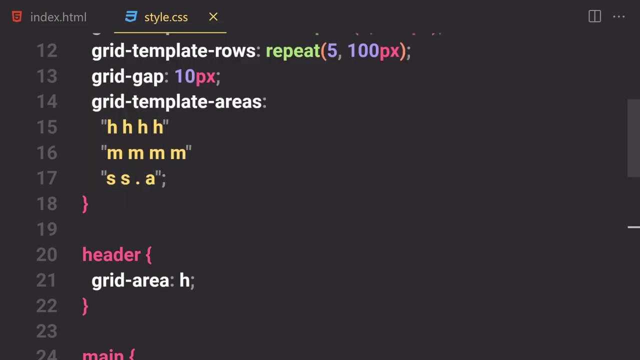 class of s and if you save that, and here you can see, this section is now taking all of this area right here. okay, something went wrong. we have our section, then we have our footer. uh, you know what? something went wrong a little bit. now let's just go to our style sheet. so we have section section. 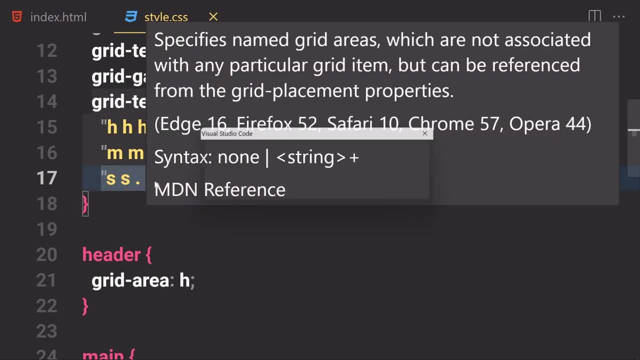 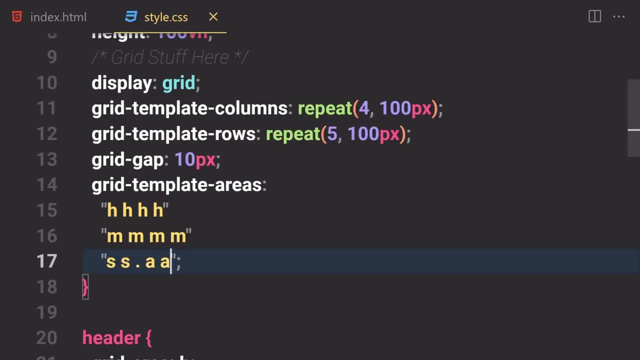 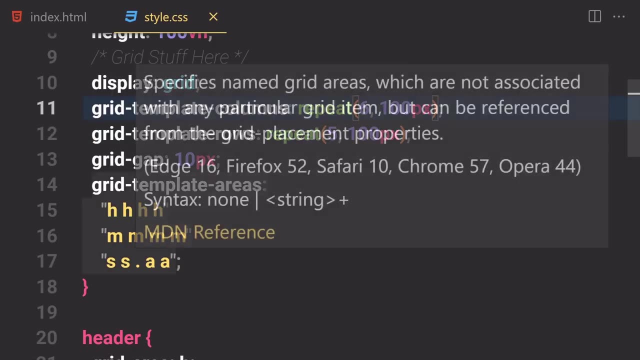 and then, instead of using this period, you know i'm going to also provide another one. okay, so i'm going to just use the a right here. if you save that, it gives us a footer. that's because we don't have enough uh, rows and columns. so if you sell that, okay, so we don't have a lot of. we have s s one, two, three, four. 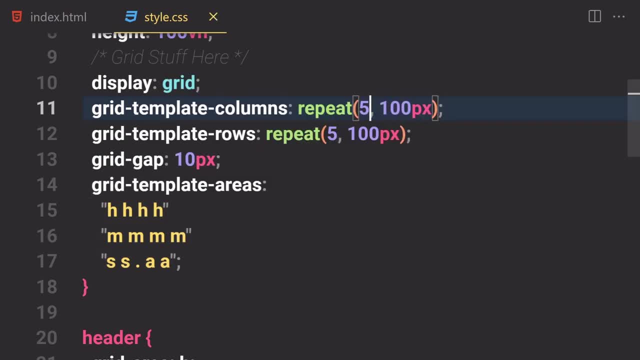 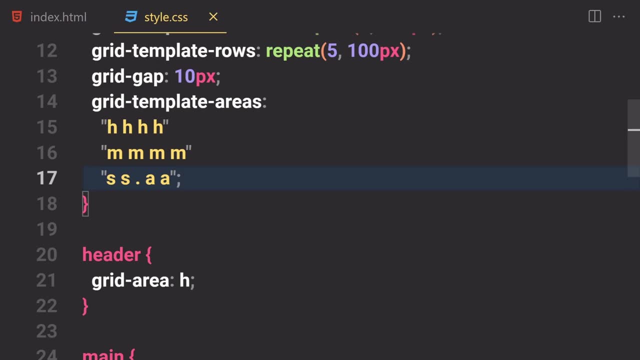 five, and we have to provide a five in there and so there. so this is going to be the first element. this is going to be nothing. and then we have a third element. so it's not showing up anything. you know, i'm going to remove this uh 1a from there and so there, and now, here you can see it will now. 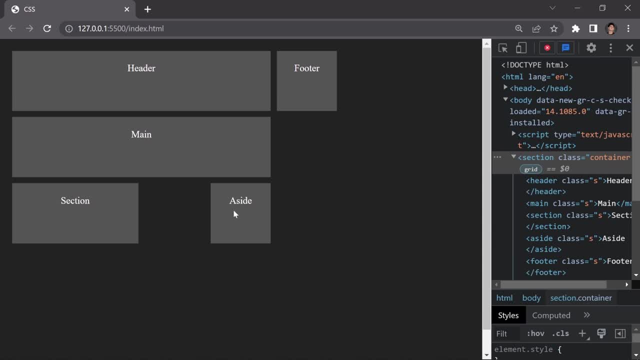 give us this section, section, and then it will give us nothing inside there and then it will give us a side right here. so instead of writing, uh, five rows, i'm going to set that to four rows. uh, you know what, i'm going to set that to like. 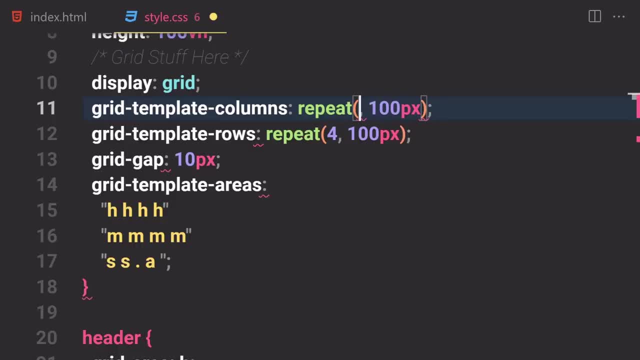 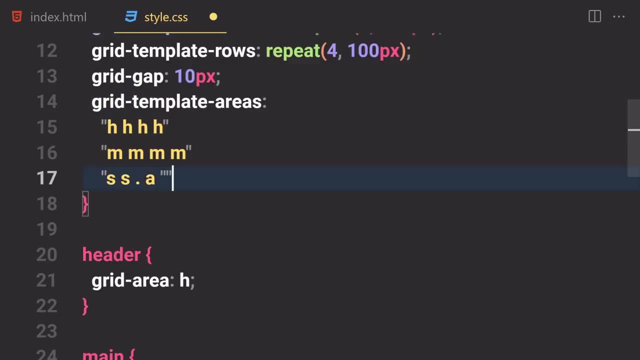 six rows columns. so we don't want six column, we want four of them. and we'll now push it right here and we don't want in something inside there. so you know what? we're going to be just selecting a footer area right here, so i'm going to just write f, f, f and f, so this footer will take this. 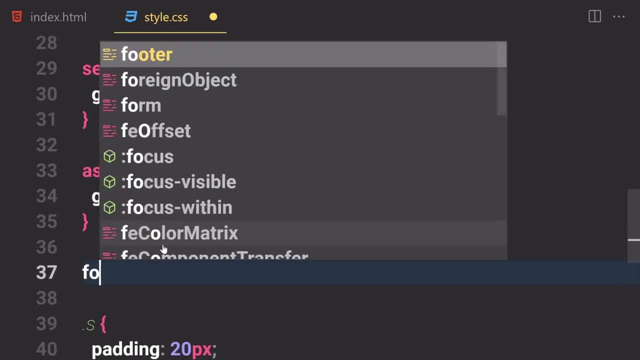 place. so we have to just specify this footer. right, here we are going to be selecting our footer, and now let's just provide a footer. and then we're going to just select this footer, and then we're going to create a grid area property for that, and here we just have to use this f, and if you 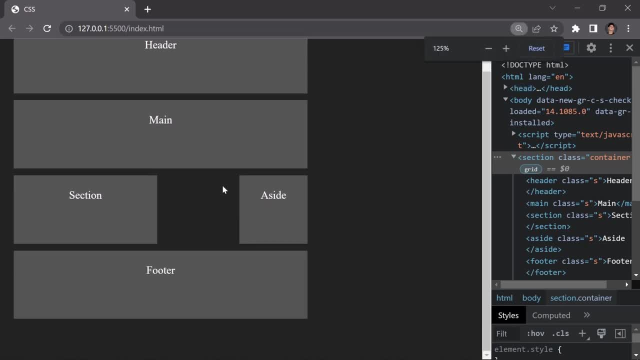 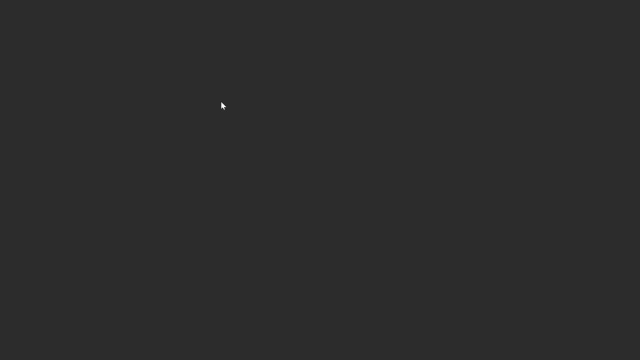 save that and boom, here you can see we are now getting this layout right here, the same like this one, not the same, it's taking all of its place. but i just kind of want to show you is that how can you work with a grid area property, and this area, grid area property, is supremely useful now. 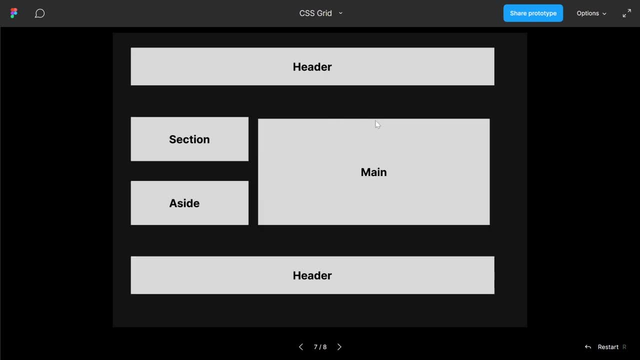 if you want to change this layout to this layout. so how can you go about doing that? well, we are going to be leaving this header right there and we are going to be first of all using a section and we are going to be providing- and- uh, what do we call it? a main area. so now let me just write a. 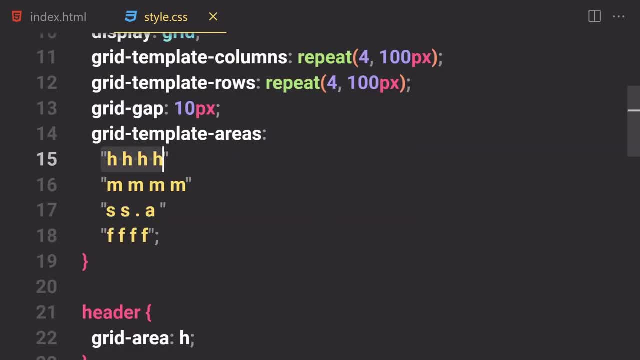 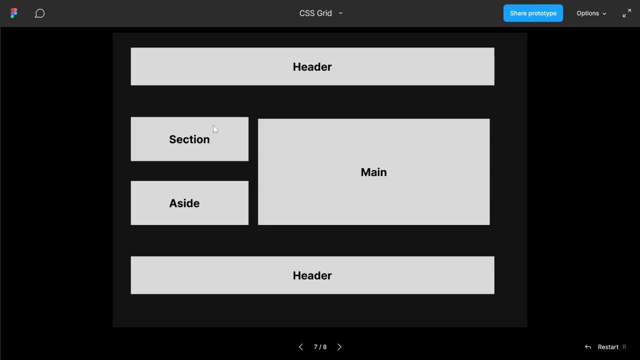 code, then you will get to know what i'm talking about. so now header will be on its own place. so now let's just use uh s right here. i'm going to put s in there, and i'm going to also put s in there, and then main will be in its own place. and now here, instead of that um ss in here we just have. 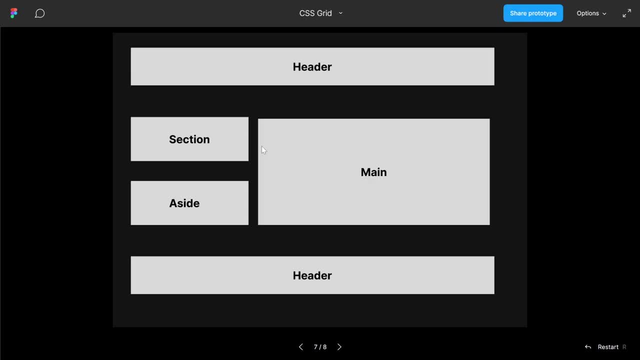 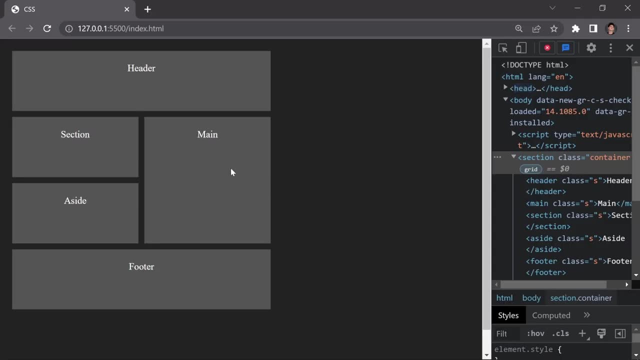 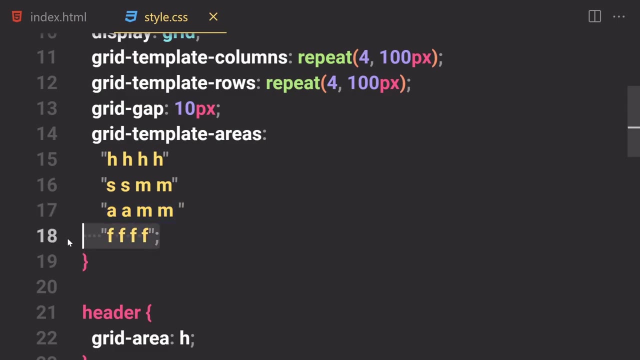 to put that like a and space a, and we don't want to put a spaces in there, so we have to just use m. so if you saw that, and now let's just check it out, so here you can see one log user section and a side right here, and our main area is now at this place right here, and our footer is also. 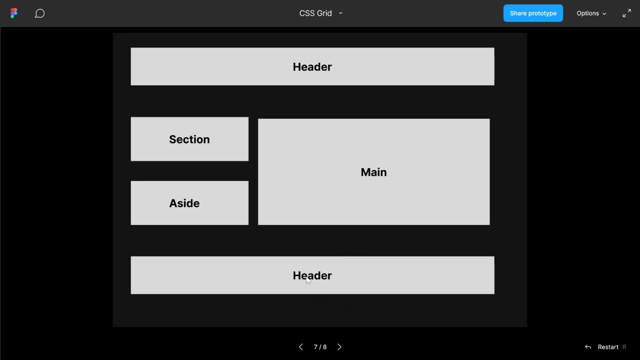 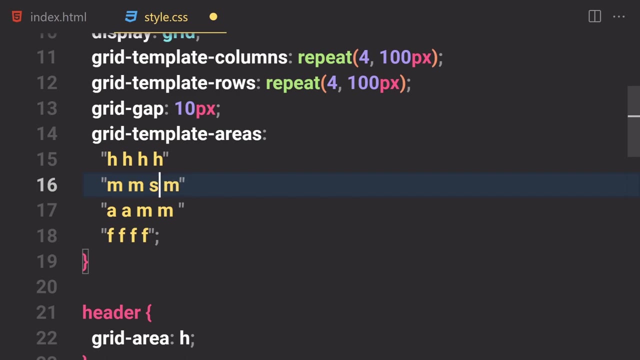 taking its entire area, like. so i should have to change the header to a footer. i apologize about that. and now, if you want to change this layout to this layout, so you can also do that by just writing m in here. so i'm going to put like um, m and m in here and i'm going to change that to. 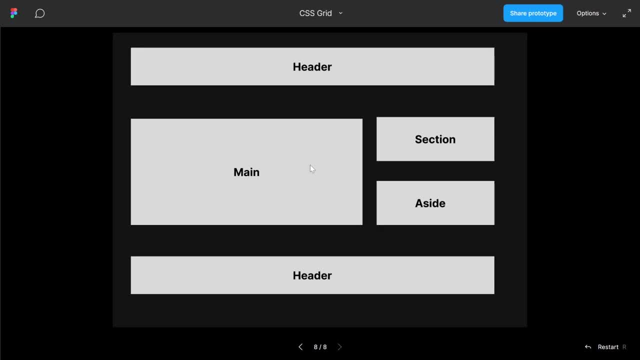 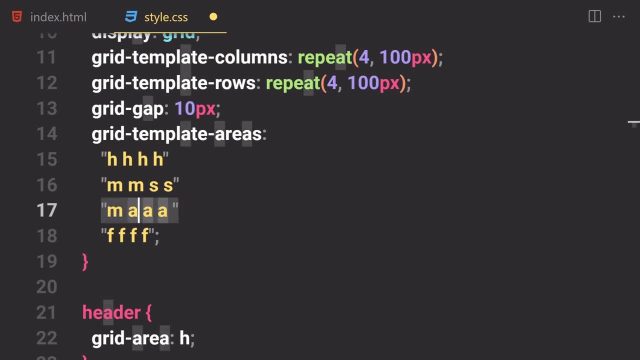 what is the section. so let's just change this one to section and then we have a side and a side. so i'm going to just write a and a in here and then m and m in here. so if you sell that, and now let's just check it out and boom, here you can see, we get this layout. 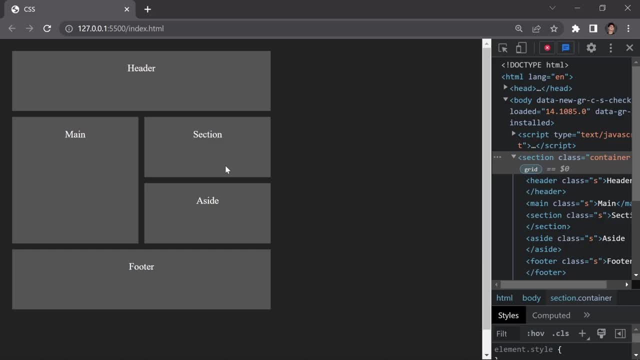 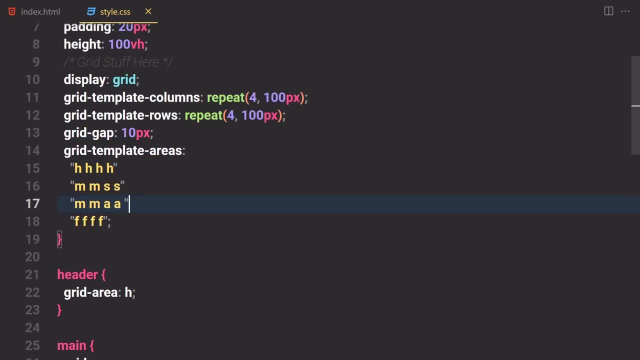 right here. so that was kind of simple to work with the css grid. and i know css grid can be a little bit overwhelming at first because we have a lot of properties and it's different kind of values and my recommendation will be to just play around with the css grid and it will just click it for. 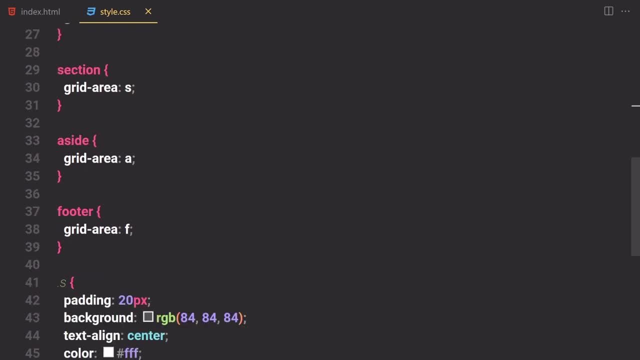 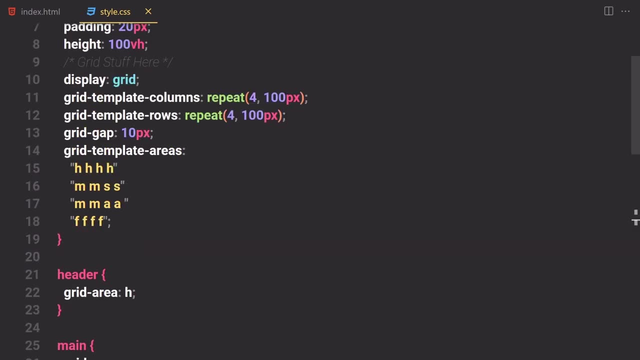 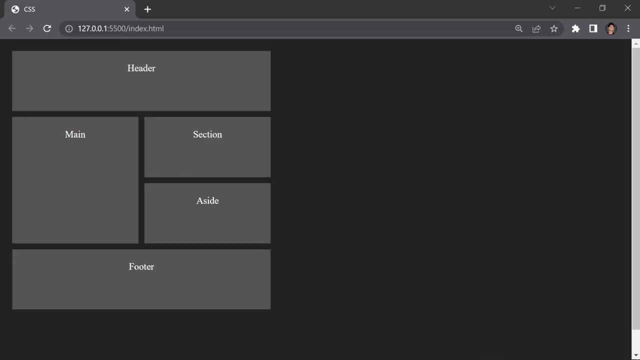 you. i know that you cannot learn css grid in one day. it will take a little bit of time to learn. so if you learn css grid- and chances are like you, maybe like 80 percent- learn, uh, how to build up projects by yourself and by using html and css anyway. so i'm going to just close that out and i 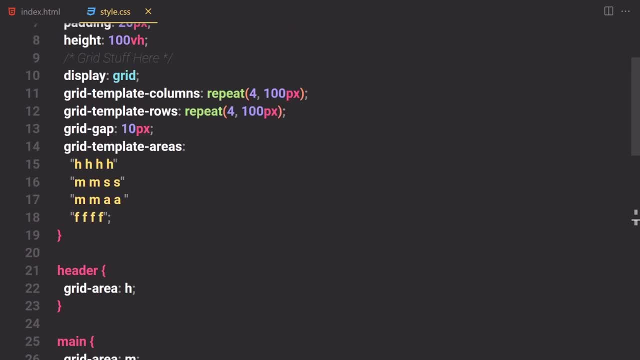 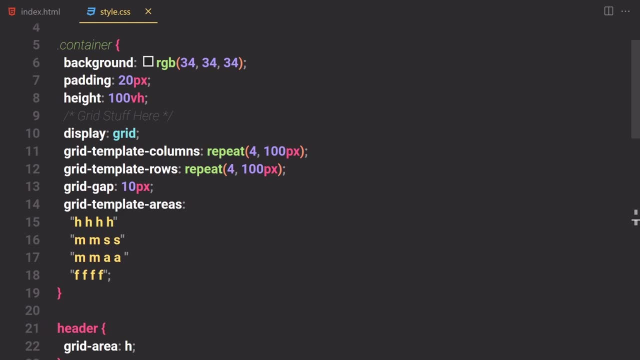 guess we are totally done with the css grid. so what do we learn so far? first of all, we learn about a display property, then we learn about grid template columns, grid template rows. we also learn about a repeat function. we also learn about gutters or gates, and we also learn about 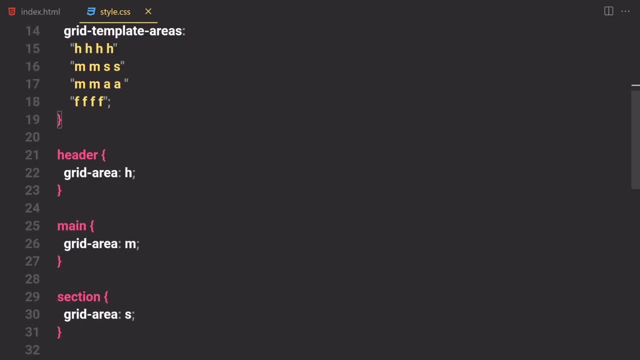 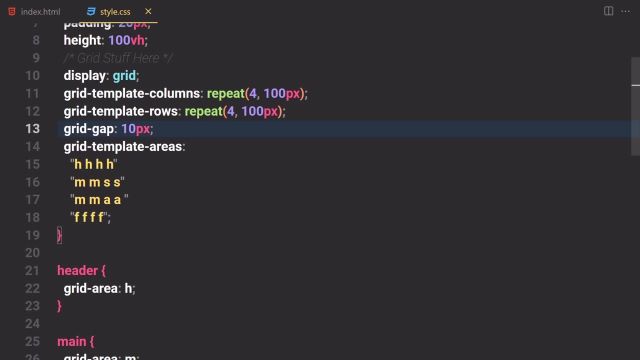 gapping, whatever you want to call it. and we also learn about justify content, align item, align self and all of that kind of property, order property. and finally, we just learned about a grid template: areas and areas are areas. areas are supremely awesome in css and i really love uh css um grid. 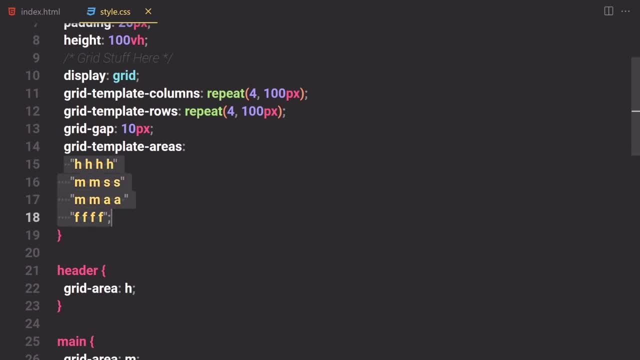 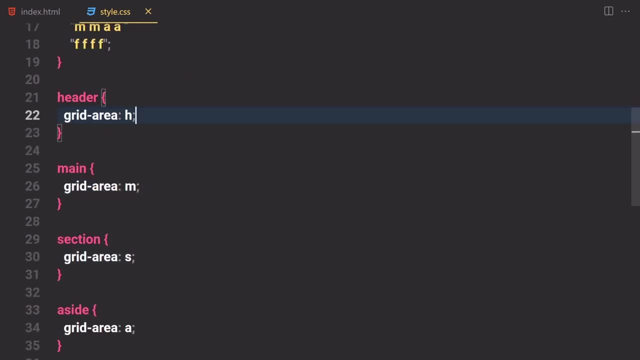 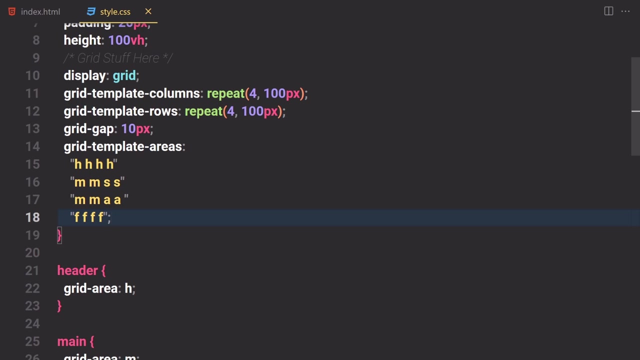 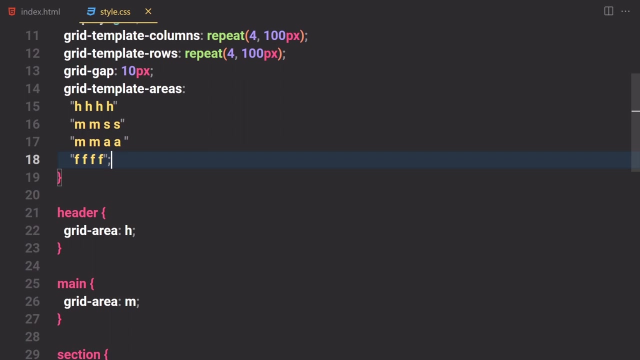 template areas. so first of all, you just have to declare your layout like how your level should look like, and then you just have to use this grid area in their specific element. okay, so that's it's part to thehow we're going to do, and that's it for today. i just wanted to give you another. 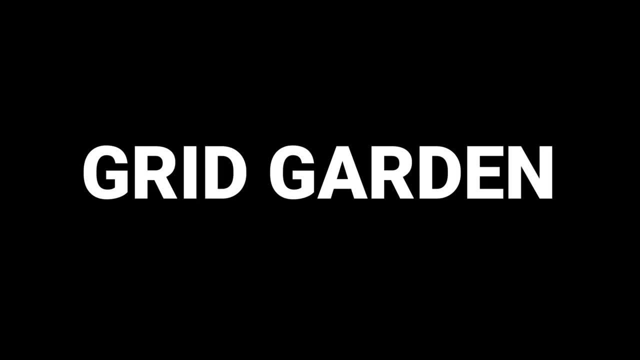 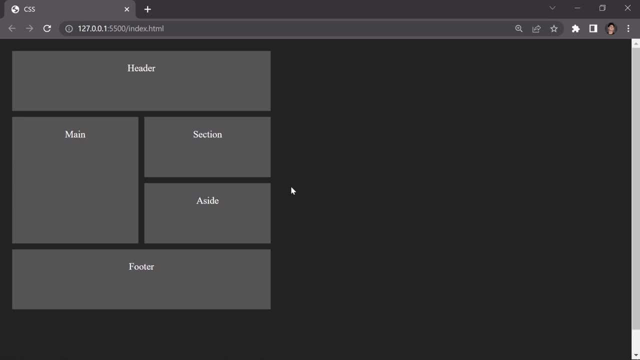 question in the chat, or maybe not, but it will just take a little bit of time for you. i promise it will take a little bit of time for you to catch up. so if you master css grid and, as i said, you, if you are not 80 there, so maybe you are more than 50 percent there to build your own project by yourselves. 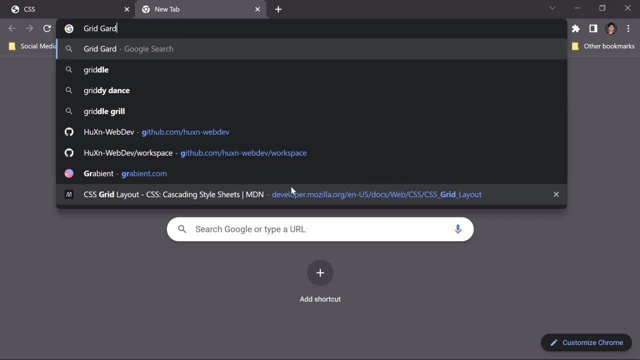 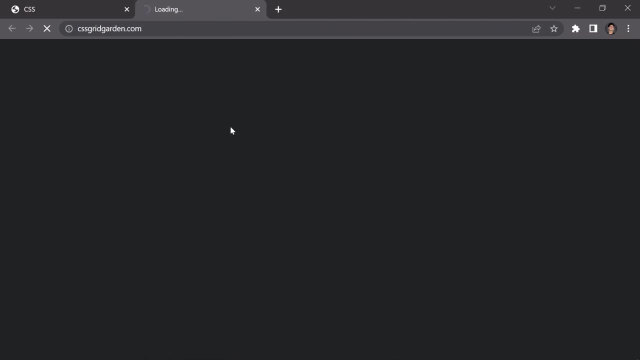 css, grid garden, i guess, uh, grid garden. so now let's just search for that game. and now, here you can see, we have this cssgridgardencom and i'm going to click on that, and now let's just play this game. all right, so what do we have? you can learn the instruction about that, but in my case, 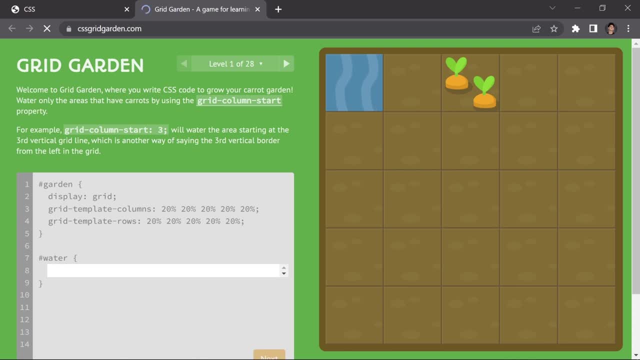 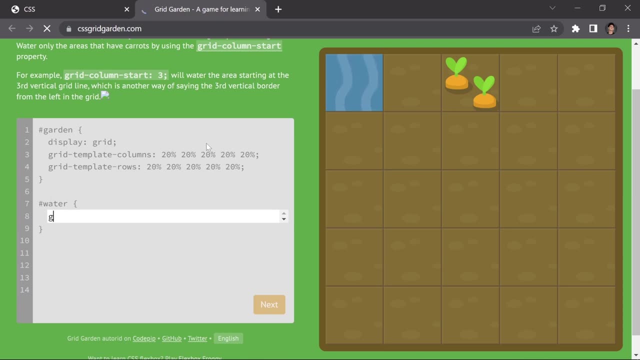 i already played this game before starting this video, so i'm going to just provide you with the answers and i'm not going to waste your time and not mine. so we have a water, so we just have a grid column and then start. so our grid column start will be from the third one. so if you put 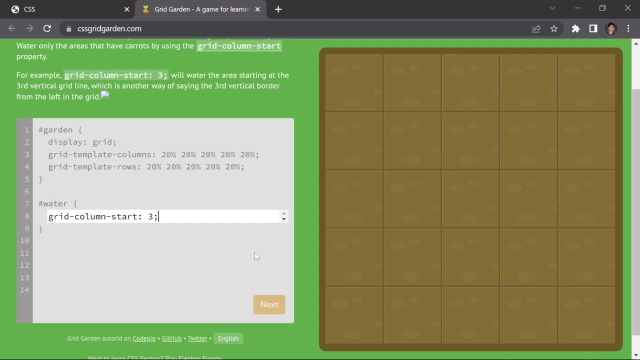 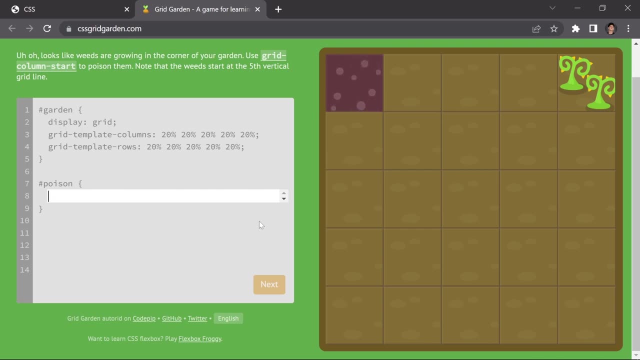 that, and now we will just push our item in there. i'm going to just give you the answers and you will play this game by yourself. i'm giving you the answer and my recommendation will be to pause this video for now and play this grid garden by yourself. and once you're done and if 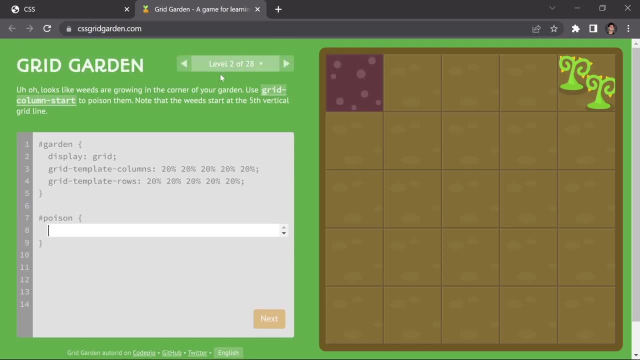 you are stuck with some some sort of a challenge, like here, different kind of levels, so if you are stuck at each level, so then kind of back and i'm going to give you all of the solutions right here and here. what do we have to do? i'm 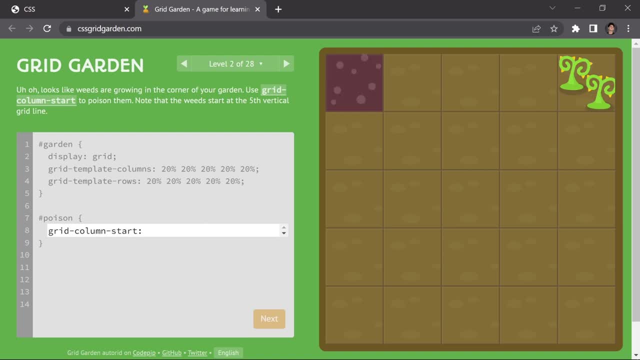 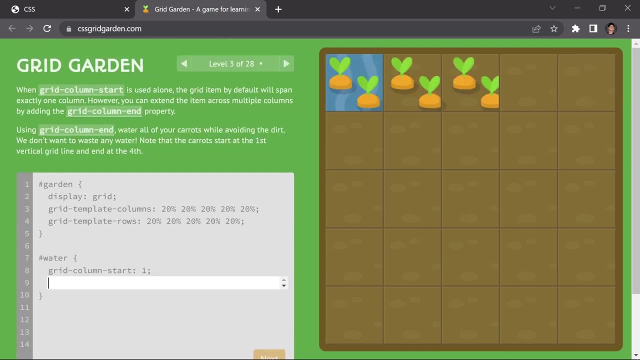 going to just put like grid column: uh, start. and as i said that i already played this game, so i'm going to just give you the solutions. if you want to fast forward, so you can also fast forward. if you want to watch the solution, so you also can watch the solution if you want to. 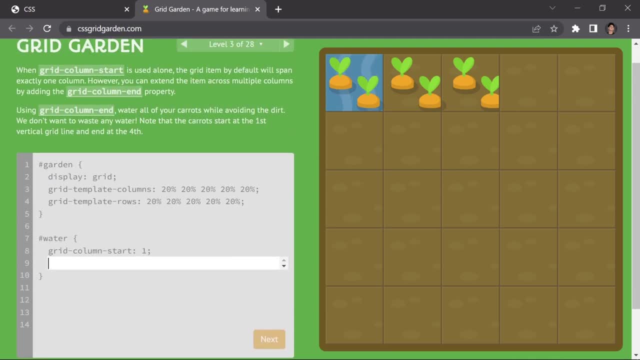 so now let's just get into the third one and the third one. what do we have to do? we just have right? uh, grid column start is already in there, so i'm going to put like grid column and then end, and here i'm going to put like four in there, okay, so let's just close that and boom, and we just have. 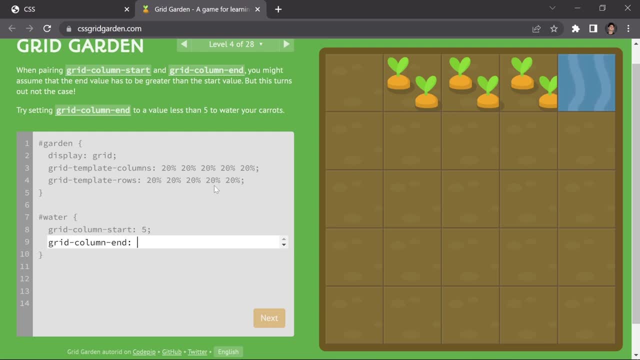 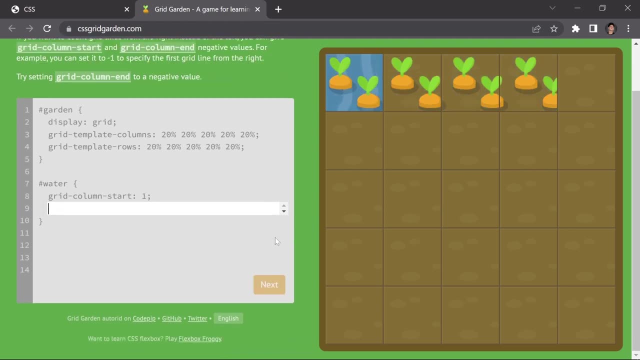 to use a grid column and and second property would be fine in this case and now done. if i start to expand each of the value one by one, trust me it will take like a different kind of course for learning about the css grid. so instead i'm going to 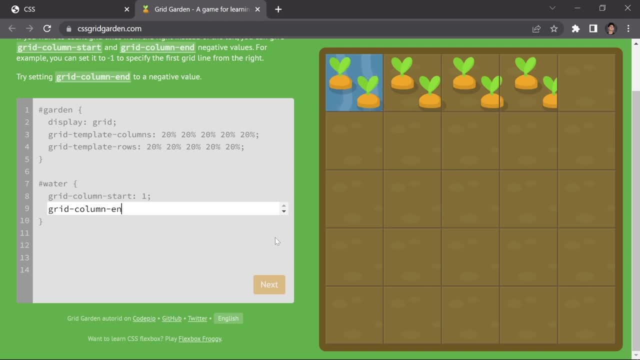 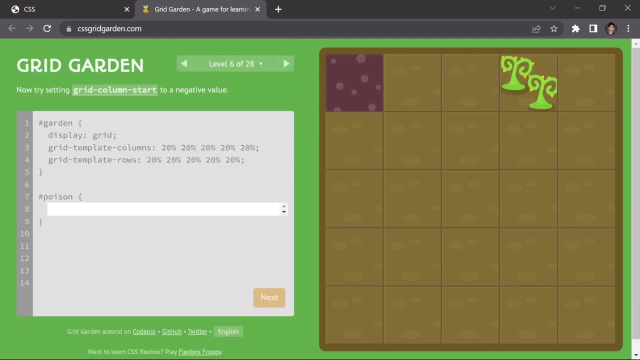 just provide you with a value, so grid column and, and, and let's just put a five in there. and if you guys want me to teach you how to play this game by yourself, like if you want me to explain each of the property, and it's ready. if i get a lot of requests from you guys, so i'm going to make a. 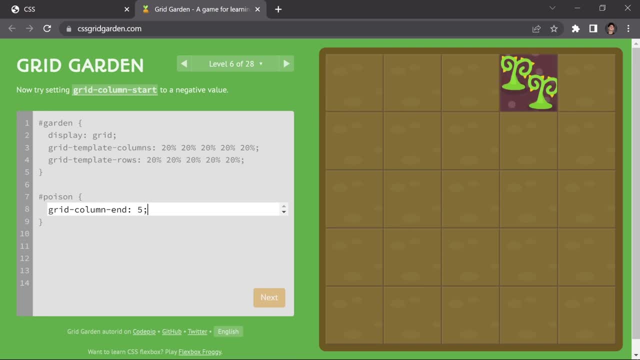 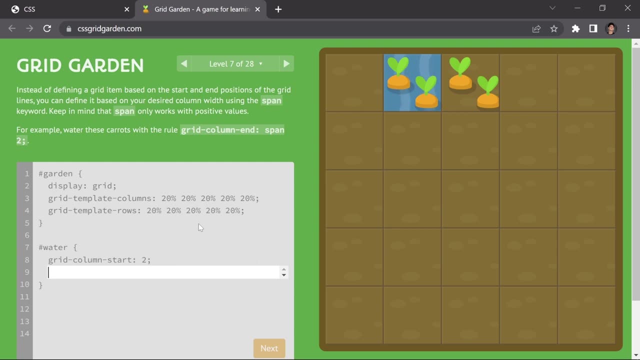 video on that. if not, so, so maybe we will just move on to a new course, and that would be fine. all right, so we are now at the level seven, and now let me just put a grid, uh, column and end and span it to the two, and span keyword is nothing special. i didn't discuss that. 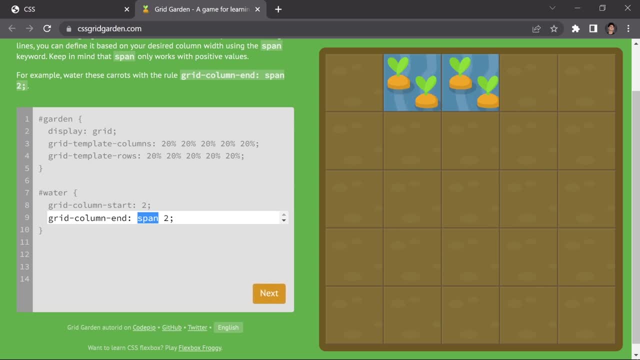 but a span keyword also allows us to spend our element and the default value is just a line which you are currently selecting your element from. so this is going to be like a flex uh or grid column start or grid column end. so the default value will be that and we can span. 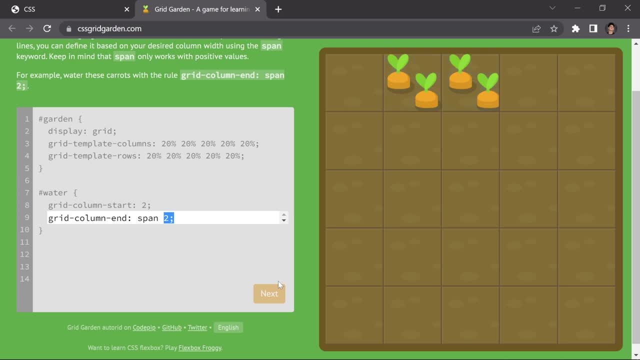 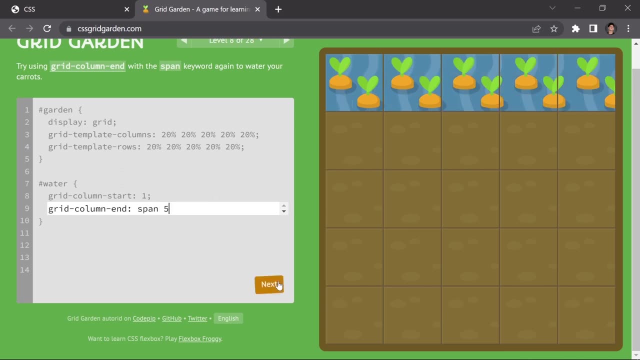 through whatever you want with that, okay. so i'm going to put next, right here, now let me just write like a um grid column and end. so i'm going to put next right here, now let me just write like a grid column, column and then n, and we are going to be spanning from whatever line we have and we want to span. 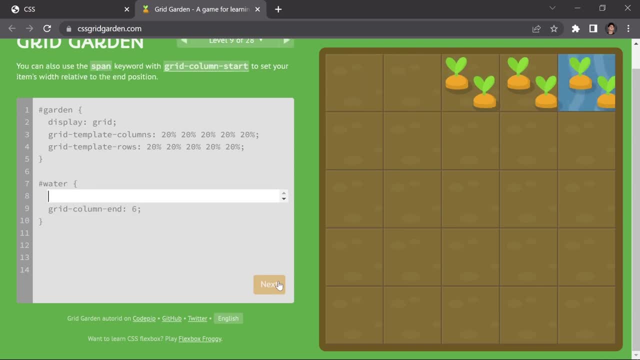 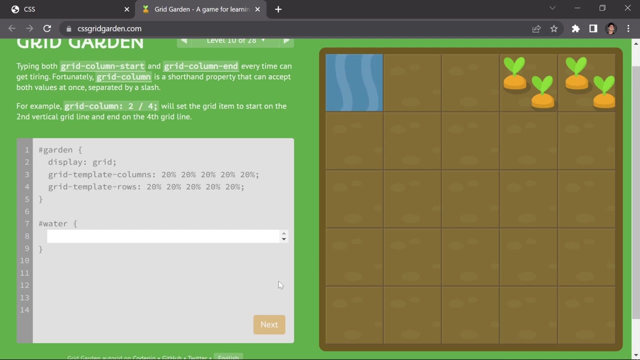 through five line. and now? now let me just provide a grid column: start and span from whatever the line is, and we want to span through the third line, okay, so that would be fine. now let's just click on next. and now, here we have to use a shorthand like a grid column, and then we are. 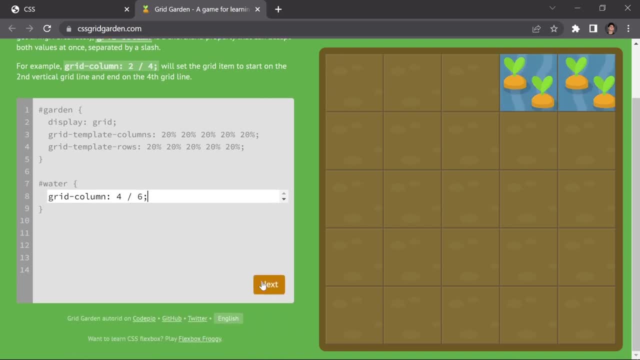 going to be starting from the fourth line and we are going to be going to the sixth line and boom, and now, in this case, we are going to be starting- let's just write a grid column- and we are going to be spanning from whatever the place is. we want to write three. 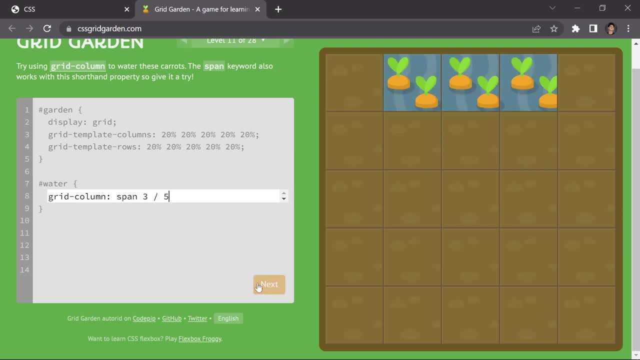 and we want to go through the fifth one, so hit next. and now, in this case, we are going to be just using like a grid row, start. it's kind of simple. so we just have right third and boom. and now let's just use our grid row. 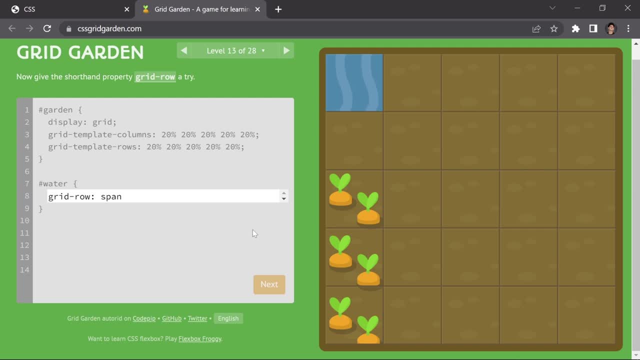 and now let's just span from, whatever the place is. Okay, so we are at the 13th, so let's just write 3 and then 6 in here, and that's going to be the solution for that. Let's just use a shorthand for writing a grid row of 5 and writing a grid. 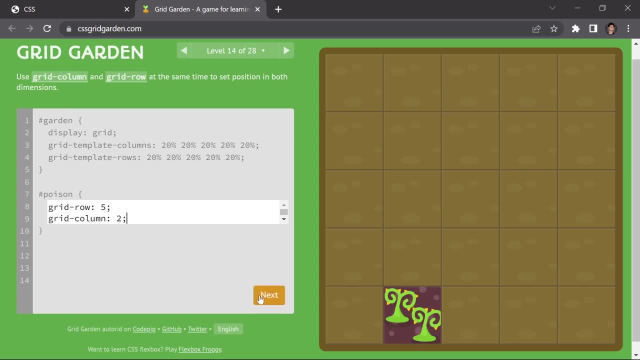 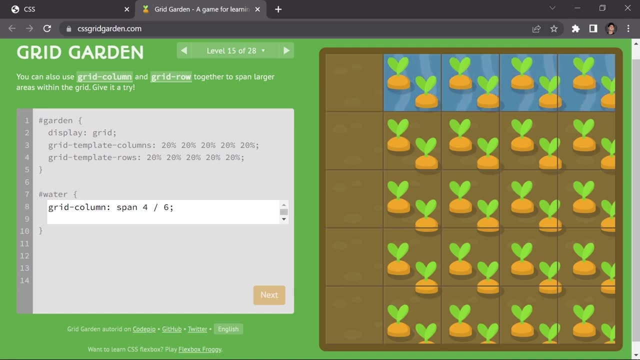 column for 2.. And boom, Let's just use a grid column span from 4, go to 6, and use a grid row of span from 5 to 6 and yep next. And I already wrote the solution for myself. Okay, I'm cheating in here. I'm not cheating. I. 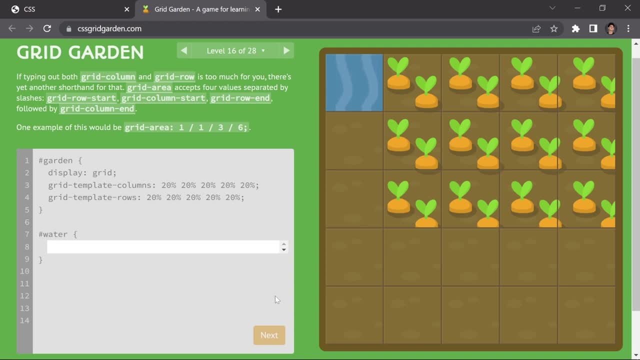 did play this game by myself, but I thought, instead of wasting your time by saying hmm, ha, hmm. so I'm going to just give you a straight solution, and I already said that you have to try that by yourself. So I don't want to waste your time and my time, so we just have to use a grid area in there. 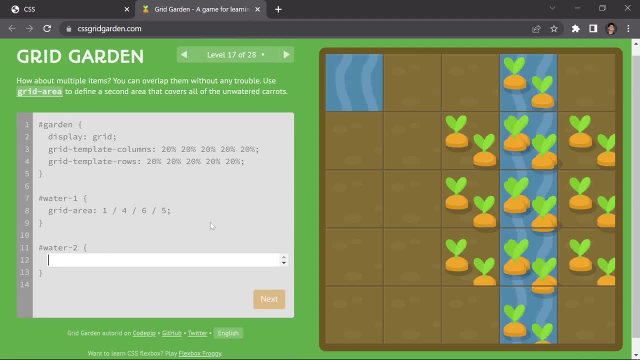 and boom, We are now at the 17th. let's just use our grid area and we are going to be writing 2 and, as I said, that grid area is going to be a shorthand for a grid row start. grid row end. grid column start and grid row. 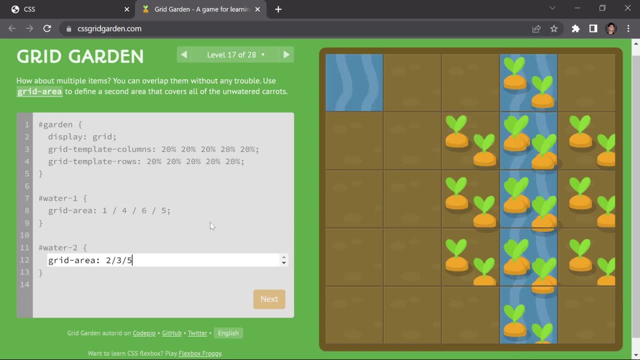 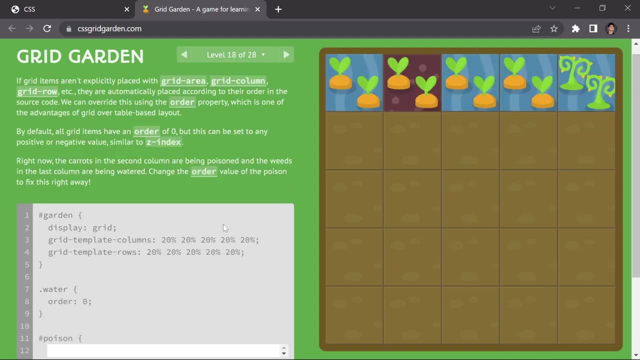 grid column start and grid column end. there we go. So, as I said there in the beginning of that, but you don't have to use this shorthand because they suck And if other developer is working on your project later, so he will be really confused by that. 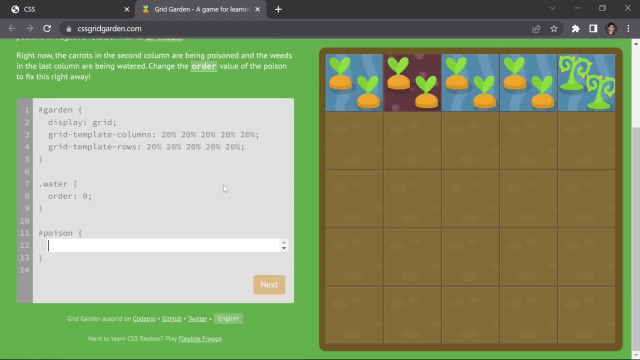 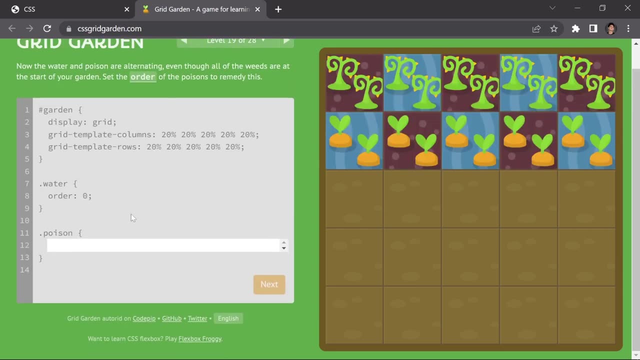 so that's why I didn't went in that much detail on there, okay, So that's why I didn't provide that much detail. so I'm going to put a order of just one we already know order and because we've learned that in our flexbox. 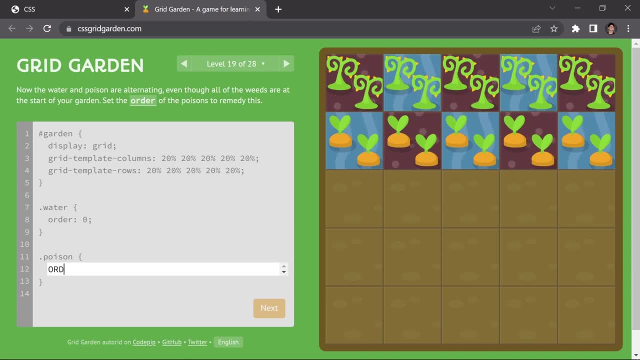 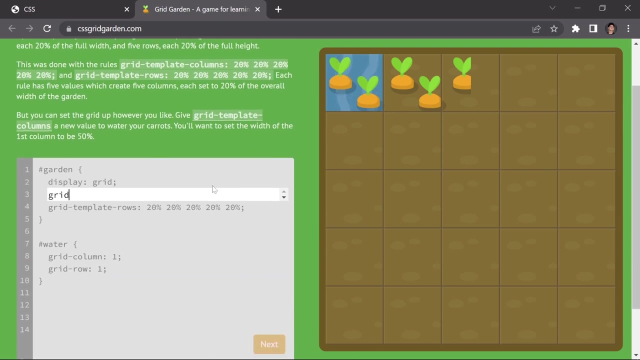 section. so what will be the solution for the ninth one? the solution will be to just use or order property of minus one and yep. next we have a 20th one. so the answer for that will be just write a grid template of rows, not arrays but columns. and here we're going to be just writing 50 and it will now take a 50. 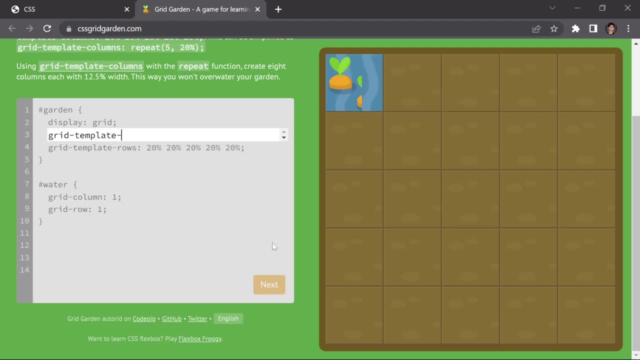 and now let's just use a grid template, template of column uh 12.5, and i know that for a fact. and now let's just close that, close it, close it, come on, close it. and now, if you hit next, it will now bring this to another one. and now in here, what do we have to do? we have to use a grid. 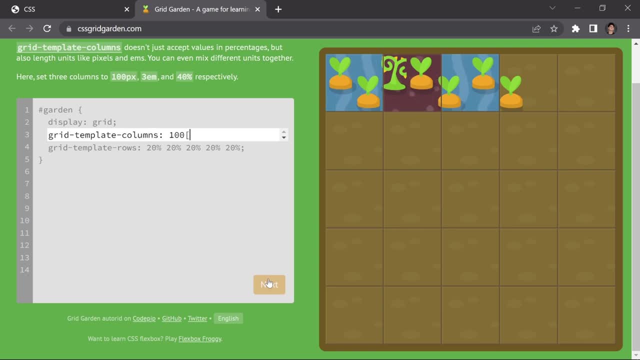 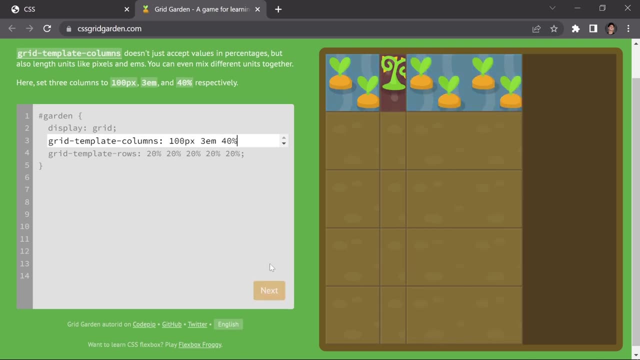 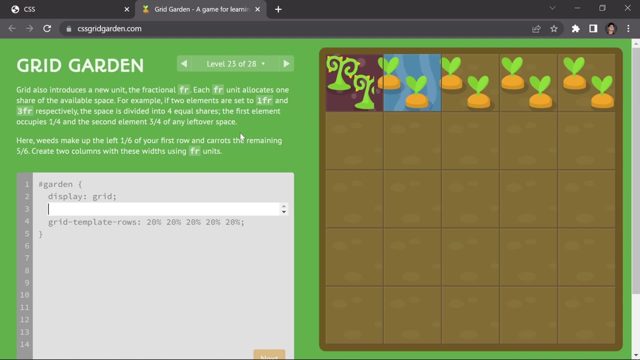 template of columns and 100 pixel, 3m and 40 percent. okay, and now, if you head next, and this is going to be the solution for 22, so now we are now at the 23 level. so now let's just uh, work on this. we are going to be using a grid template of columns, columns, and now let's just 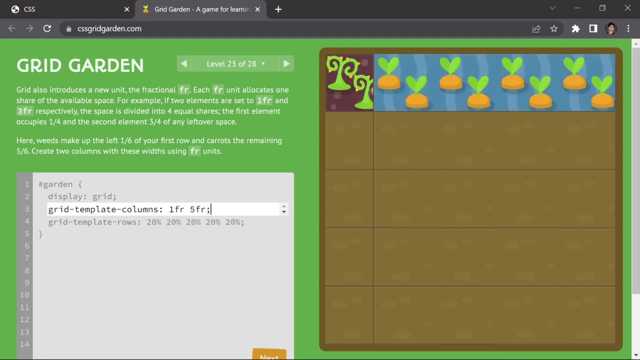 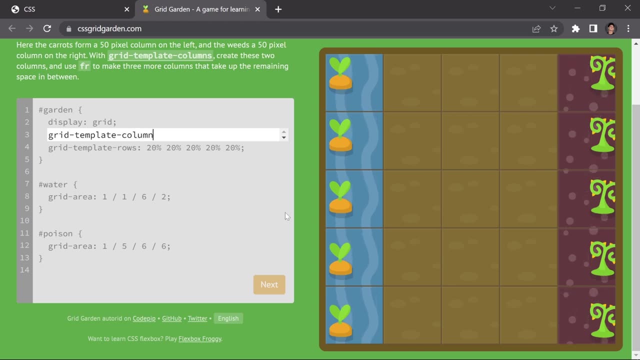 use one fr like a fraction and then five fr for the fraction and yep, that's correct. the solution will be just a grid, template columns and 50 pixel: one fr, one fr, one fr. or you can also use a repeat, uh repeater, and first of all the value will be like three, and we can also provide. 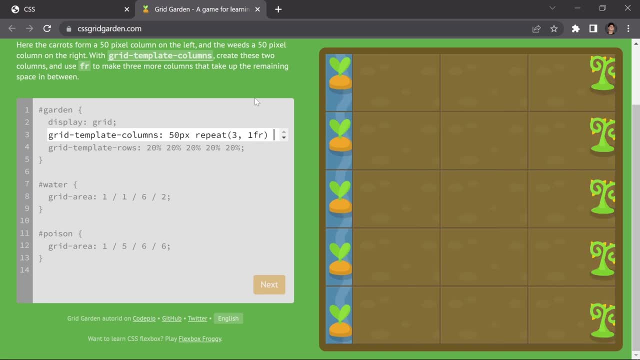 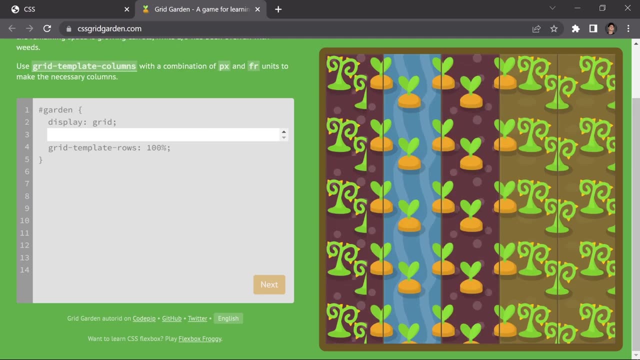 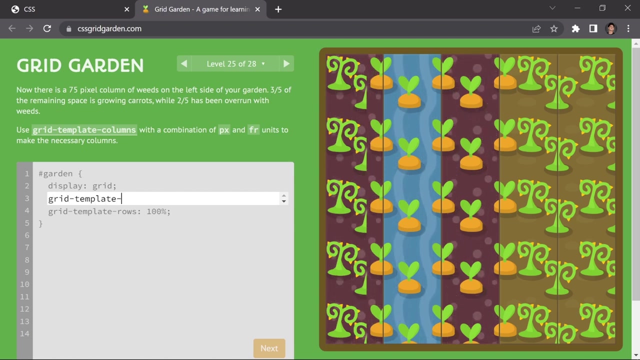 like, uh, one frs in here and we can just write a 50 pixel in there. so this is going to be the solution, or you can just write one fr, one fr, if you want to. so now, what would be? we are now at the one. so the solution for this one will be just write a grid, template columns and 75 pixel. 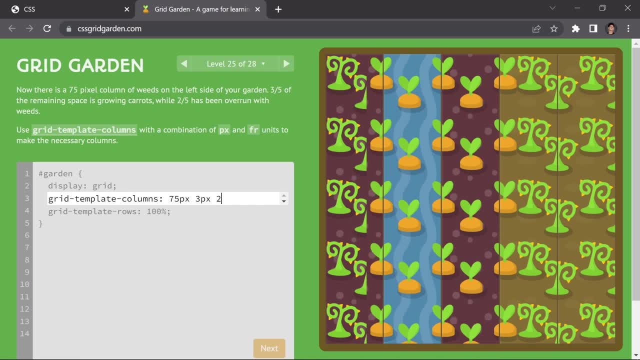 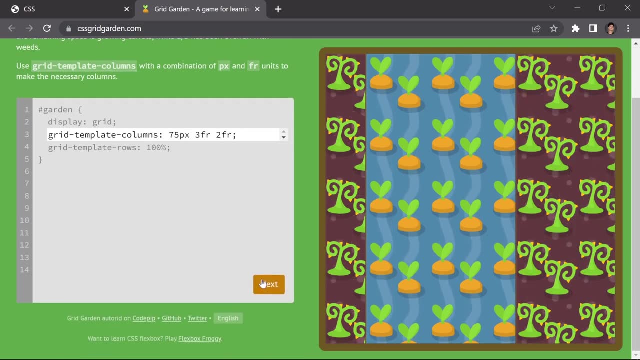 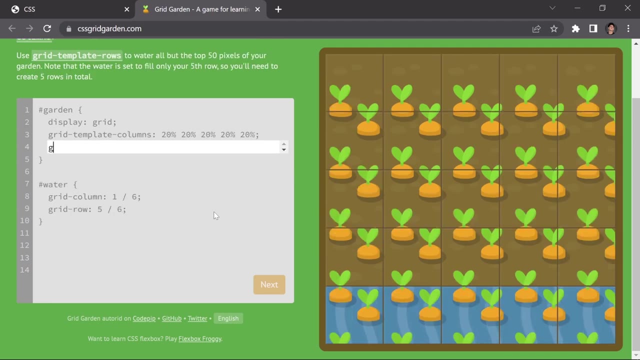 75 pixel, then we have a three pixel, and then we have not a pixel, to be precise, but we have three fr and then we have a two fr. okay, so this is how everything should work, and now let's just work on our 20th six one. so the solution for 20th six one will be like a grid template are not column. 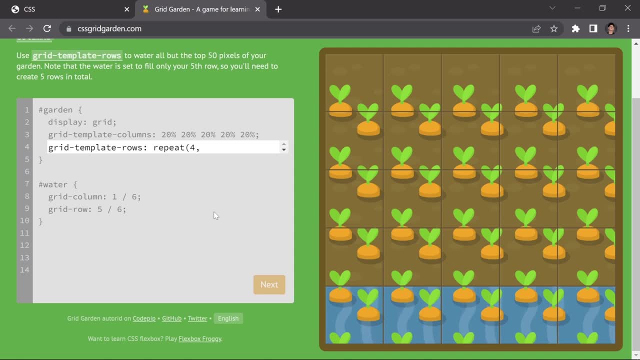 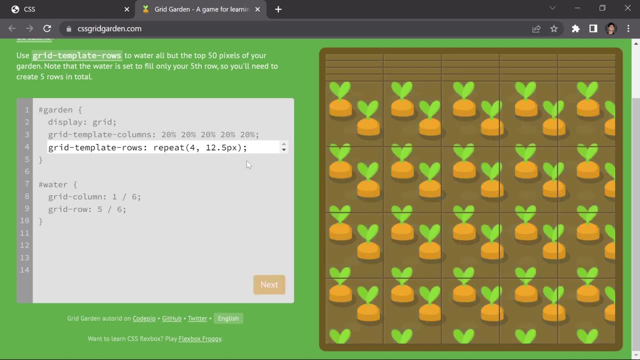 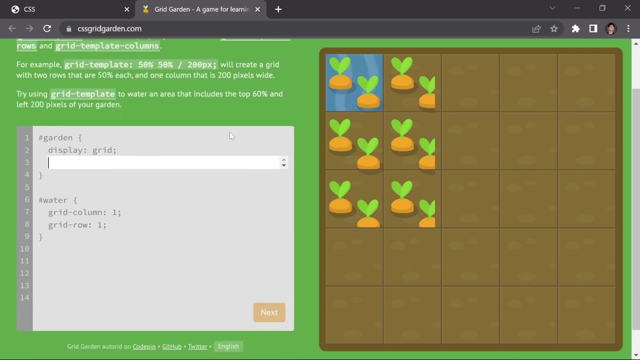 and repeat function. we can just use four 12.5 pixel. you know that for a fact. you know it's like 12.5 pixel and now let's just work on. i guess this is the fun. no, it's not a final one. we have still. 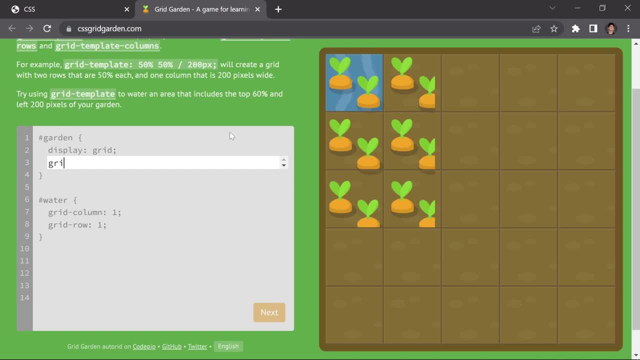 have one more left, so you can just use. and i didn't show you that, i apologize, so now let me just show you that real quick. so, templates: instead of writing grid template, columns and grid template, we can also use grid templates. so, uh, first of all, we are going to be writing a value for the. 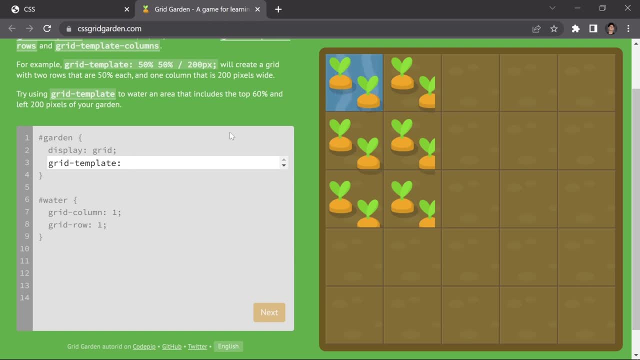 column and then we are going to be using a value for rows. so we are going to be writing, uh, 60 percent, and also 60 percent- let me just write a percent in here- and then we have to provide a column value for that. you can learn more about this grid template property, but my 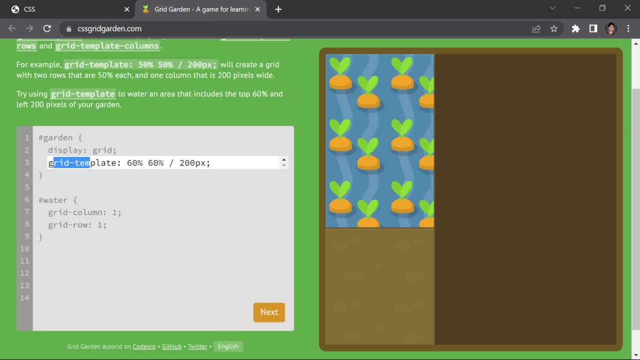 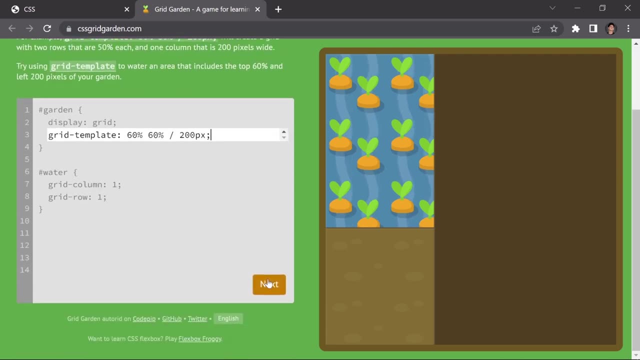 suggestion would be to do not use a grid shorthand property because it confuses a lot of people, like in. some people will be coming from a background of a back-end developers and they won't understand, like, what is a grid template and they will waste a lot of their time just figuring out and they will 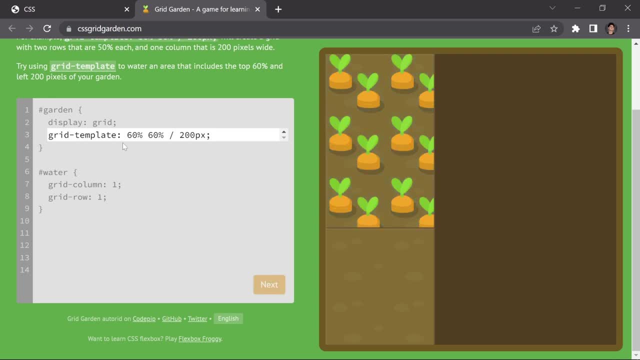 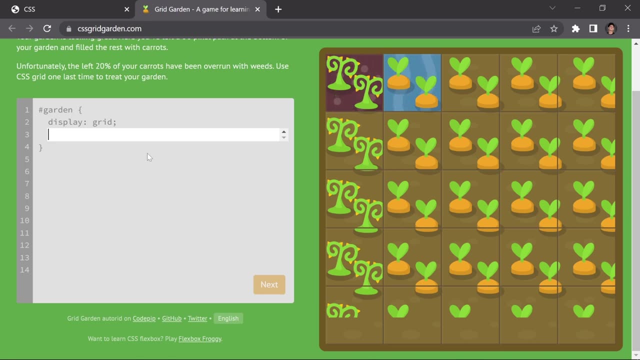 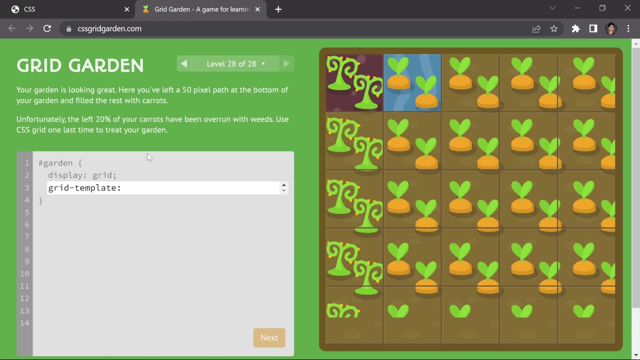 be all the day on a stack overflow post like: what is a grid template? okay, so instead of writing just a grid template, you can use a grid template uh, row and grid template columns, so you choose whichever you like, and then the final solution we have is a grid template, and then we have to use a. 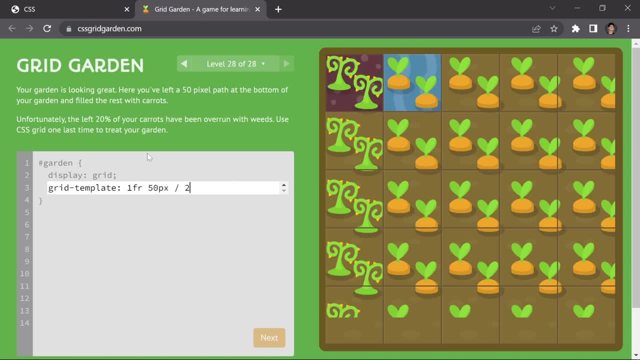 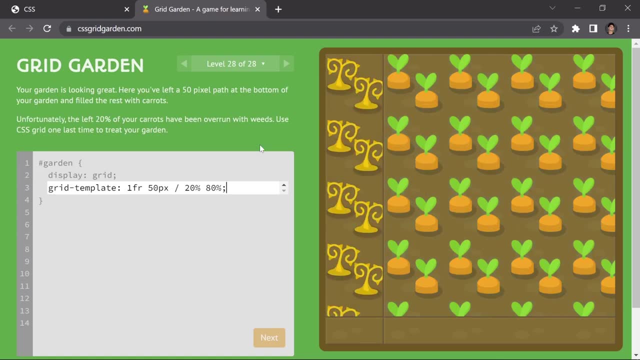 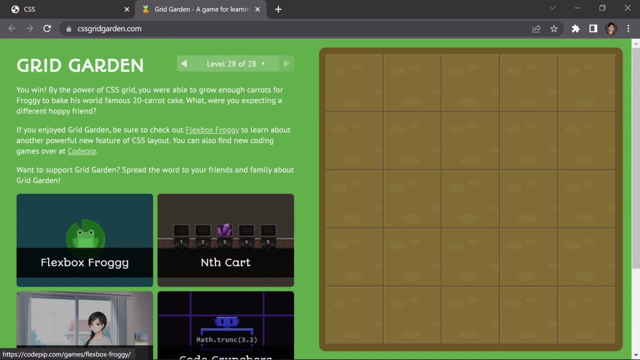 one fr 50 pixel, and we have to go through 20 percent and also 80 percent. okay, so now, if we hit next and boom, congratulations, we are totally done with our project. have you already played this game like flexbox froggy? and we already played this one css garden, and we're not going to be. 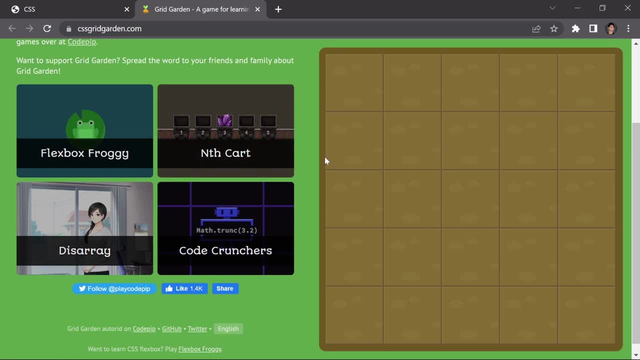 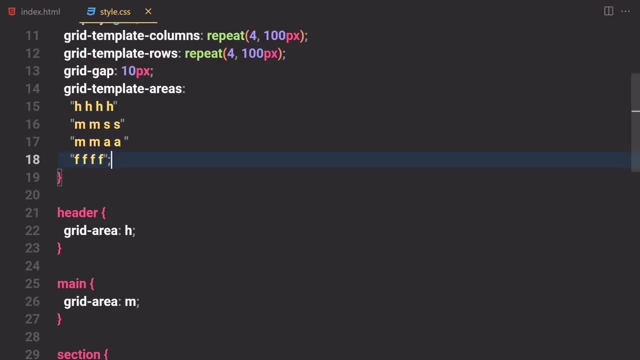 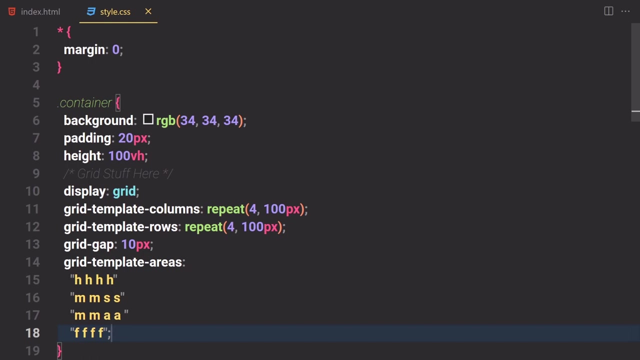 playing any more games. i guess we will. i'm not sure, but i don't know. i can't say that for sure. if you want to play these other games, so you can play these other games if you want to. okay. so that was it. a lot about a css grid. so we are now totally done with the css grid side. 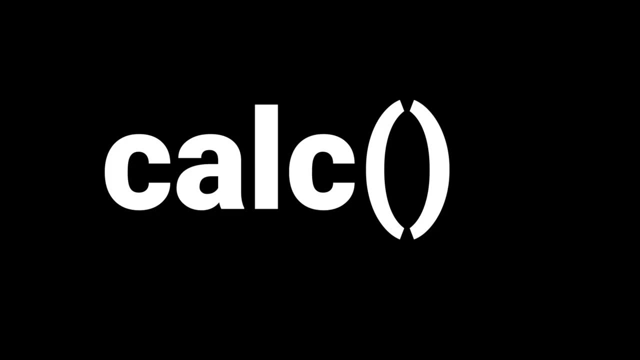 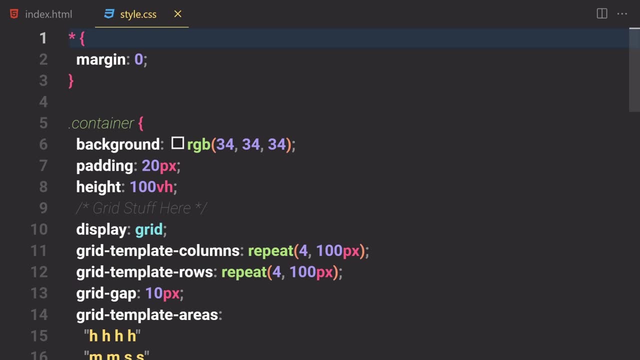 and i don't know what we are going to be learning in the next section. all right, guys, so now we are totally done with the css grid side of this course. so now the next thing which we have to learn about in css is something called a impact function. 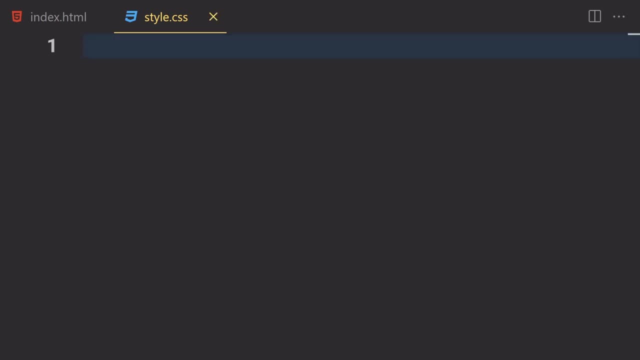 in css. so what i'm going to do? i'm going to just select everything and i'm going to remove that and what else. so just remove this section and stuff as well. so inside our body, what do i have to do? i'm going to just create a div with a class of s and no content, nothing inside there. so now let's jump. 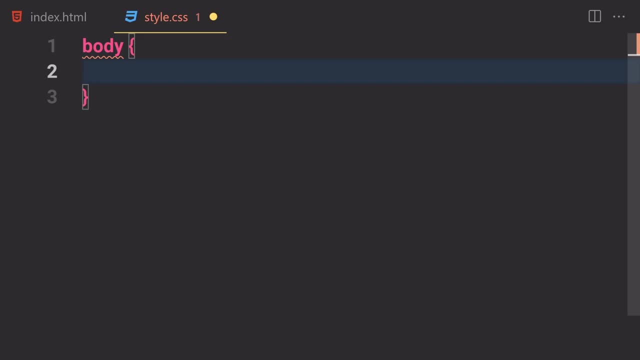 into it. but before we do, first of all we have to select our body and we have to center everything. so for that we are going to be using display of legs, justify content of center and also align items of center. okay, so now let's just start working on that s class which we just put inside. 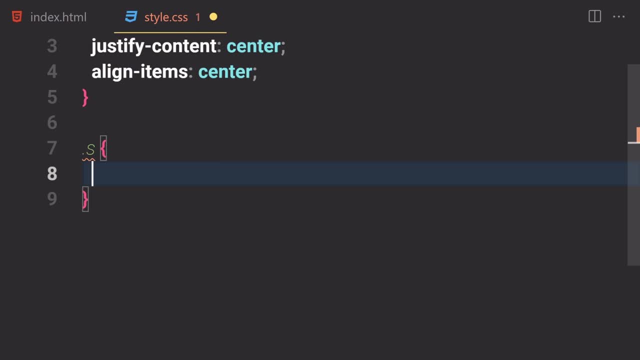 our body right here. okay, so we are going to be first of all selecting that and then we are going to be just using a bg of crimson right here, and if you save that, nothing will show up right here, because we don't have any content, we don't have any background color, we don't have 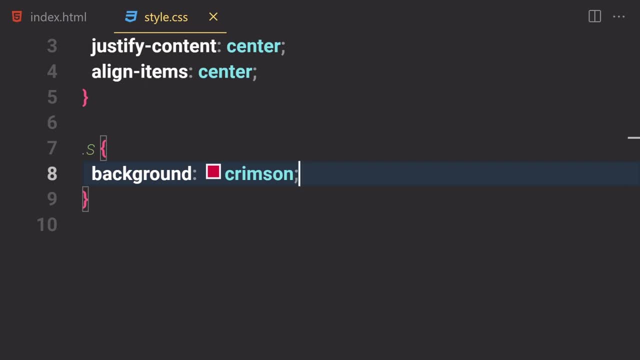 we do have background color, but we don't have any width and height and stuff like that. all right, so what is a kalk function? so a kalk is a built-in function in css and, as its name suggests, that it allows us to do calculation of our values. 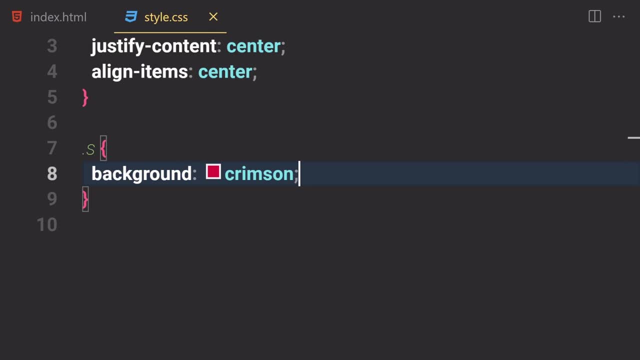 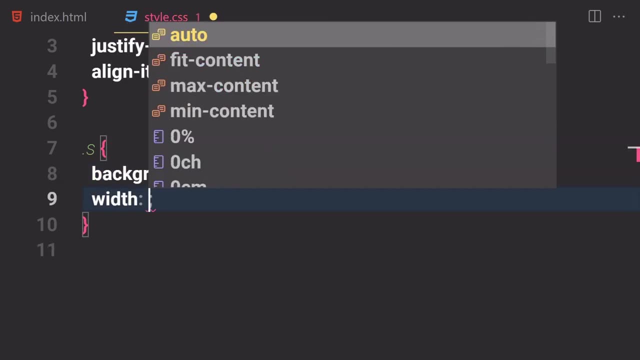 and a kalk function is a built-in function in css and, as its name suggests that it allows us to do function, just accept a few arithmetic operator like addition, subtraction, multiplication and division. so before getting into the detail of that, first of all let me just write a width in here. 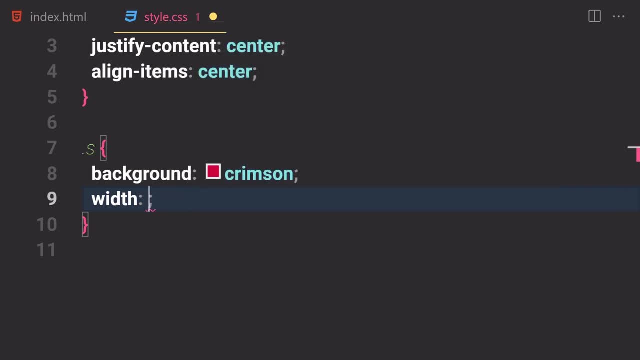 so we can just write like 100 pixel and 200 pixel and stuff like that. and now, in this case, we are going to be just writing a calc right here and now. calc will allows us to just calculate the values. so we can just write like: i don't know, we can just use addition operator if you want to. 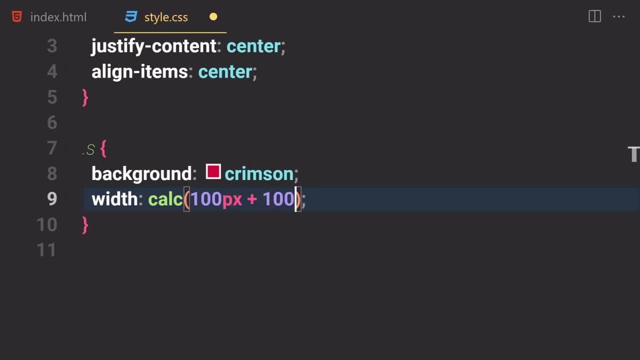 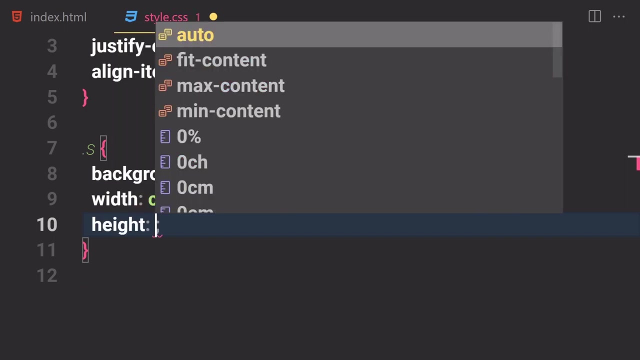 so i'm going to just write like 100 pixel plus and then 100 pixels. if you say over there and we cannot still see something. so trust me on that, if you use like plus, it will give us the result of 200 pixel. okay, so i'm going to just remove there real quick. and now let's just use a height, right? 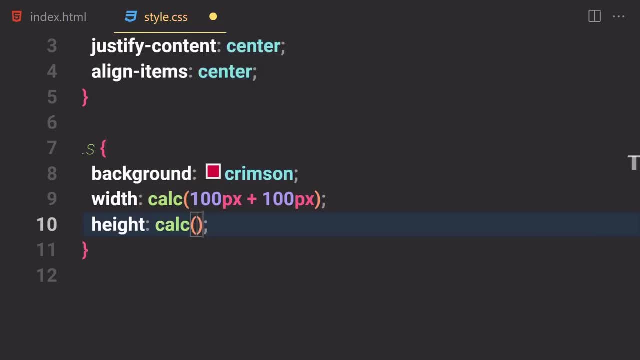 here. so i'm going to also provide a calc in there. and so what do i have to do? i'm going to just write like 100 pixel minus 50. so what will be the result? so it will just give us like 50 pixel, okay, so 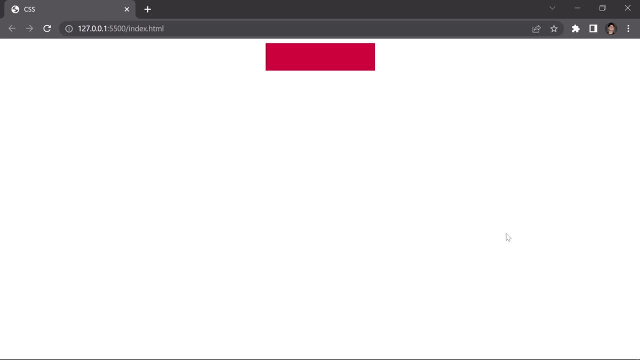 100 minus 50 will give us 50. and if you say over there and now here, you can see, we are now getting this kind of a shape right here. okay, so like, the width will be 200 pixel and the height will be just 50 pixel. so let's suppose, if i just remove 20 and if you say over there, so it will now give. 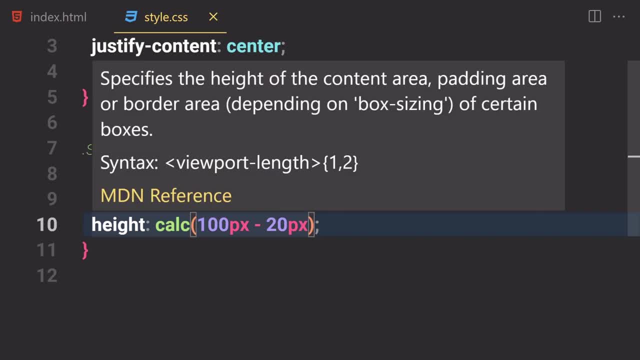 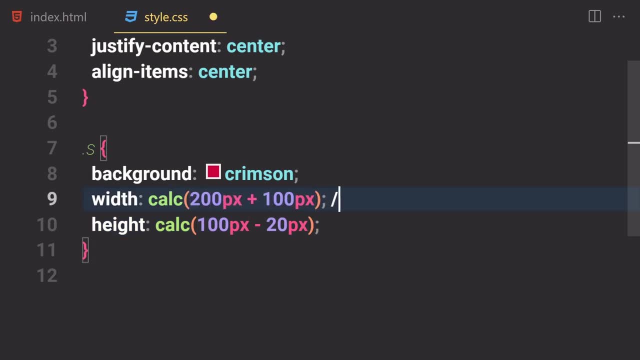 us what so 120 minus 100? so it will give us 80 pixel, and we can also increase or decrease the sizes. like maybe, i don't know- so it will now give us the result of like 30 pixel- uh, not 30, but 300- and we can also increase or decrease the sizes. like maybe, i don't know- so it will now give us the. 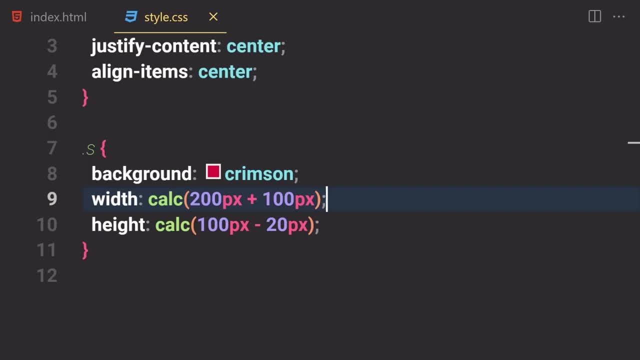 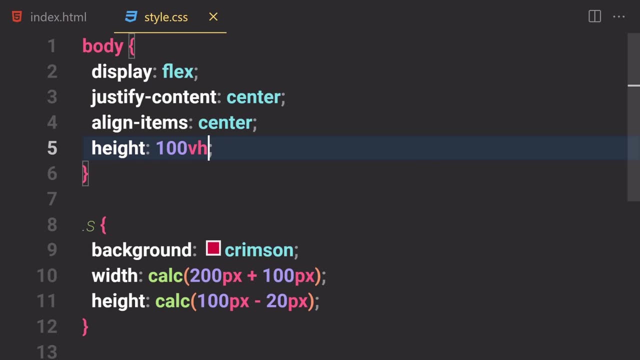 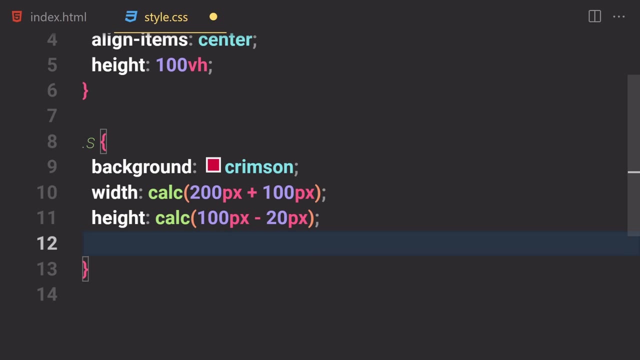 result of 20 tietheq. it will increase or decrease the sizes. okay, so, finding this particular freaking size and we can see that some more Kolk is here, and i'm going to just bring down our, my volume here, here, our volume. if you put it standing this over here, it will be about 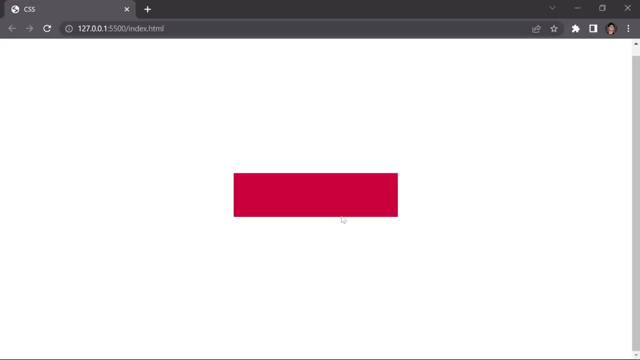 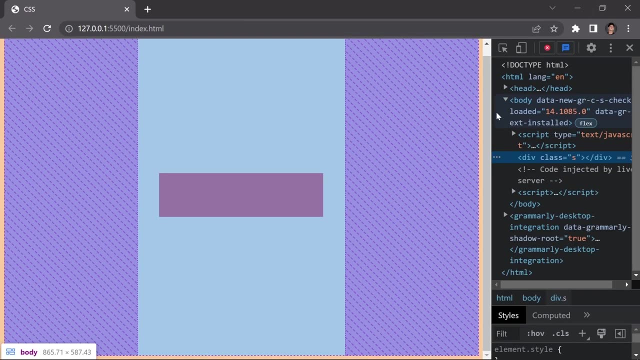 227, so it will actually separate this. and if you say over there i'm like going to put itili, you know what, if you just right click on there and if you go to inspect and let me just show you the box model real quick so i can show you that, and now here you can see the log. uses 40. 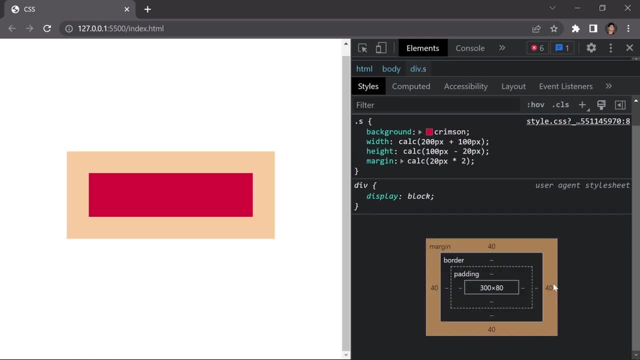 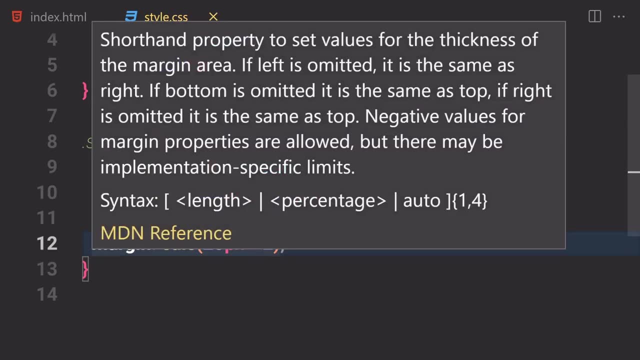 pixel to the top, 40 pixel on the bottom and 40 pixel on the left and on the right right here. okay, so it really gives us margin of 40 pixel all around, and this is using a times operator or asterisk, or whatever you want to call it. okay, so now that we learned about addition, subtraction and 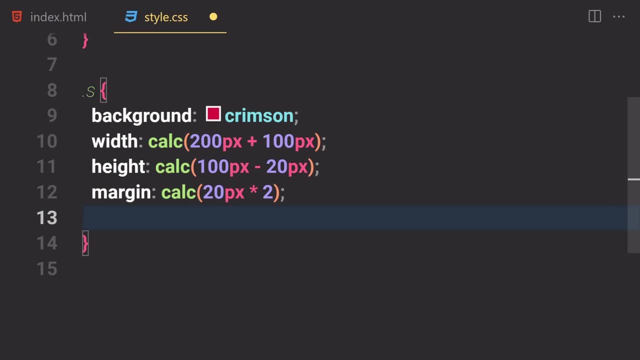 multiplication. now let's just learn about um division operators so we can just use like division operator like: so i'm going to just write a border radius right here, and we have to just write like 15 pixel first of all, and then we can use our col function right here. so 15 pixel and 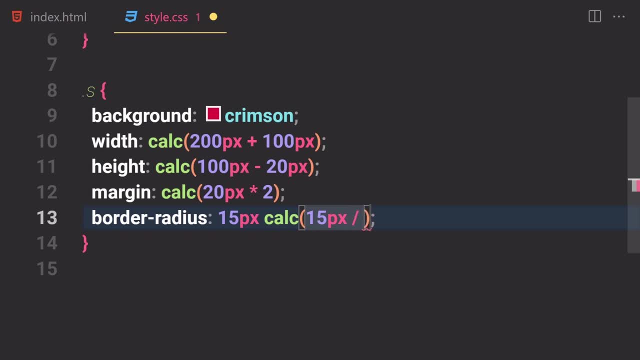 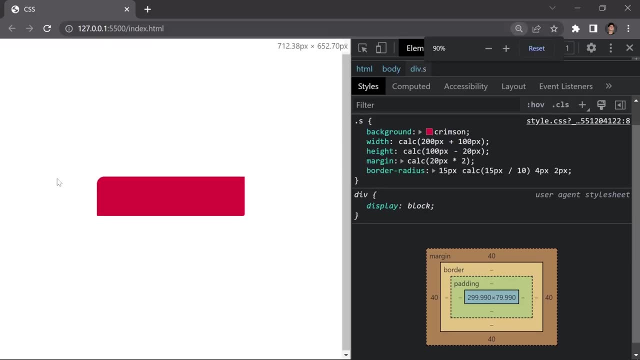 then let's just use our division operator. okay, so 10 pixel divide by 10, and then we can specify our own new values, if you want to. so if you save there and now here, you can see that it will now gives us these radius right here. so this is how we can use a division operator. so now let me just give you 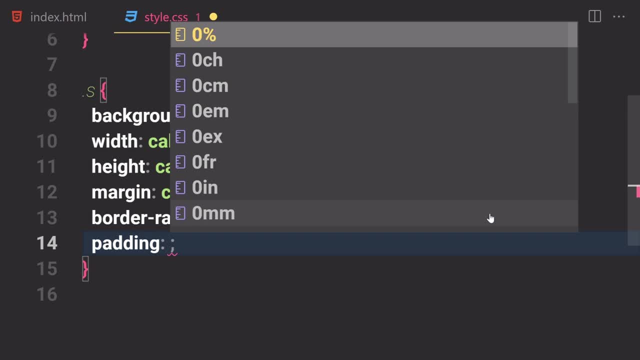 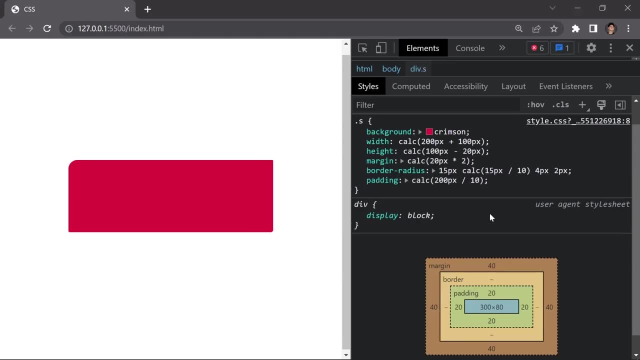 one more example of that. so if you want like padding in this case, so we can just write like a call function and 200 pixel divide by 10. so if you save that and here you can see, it now gives us that much padding right here. okay, so padding will be 20 pixel all around, right here. 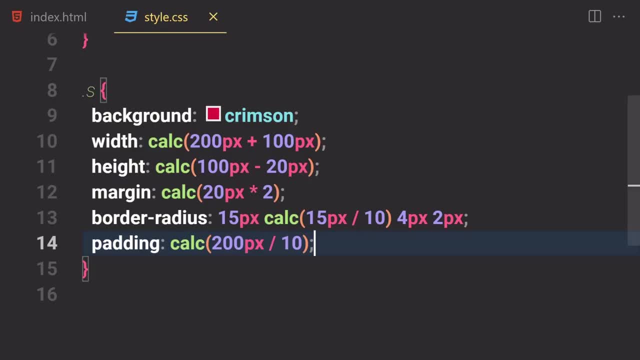 so 20 pixel top, bottom, left and right. so this is how we can use a call function. it's not scary, it's not crazy, but this is how we can use a call function. so remember that call function allows us to do calculation of values and it uses a basic arithmetic operator like addition. 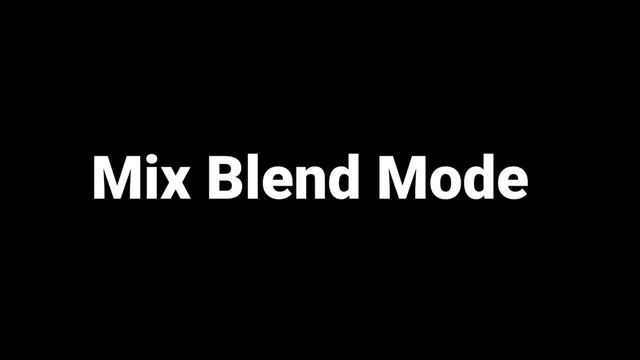 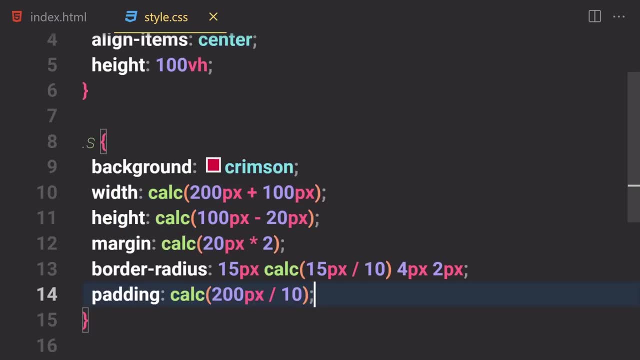 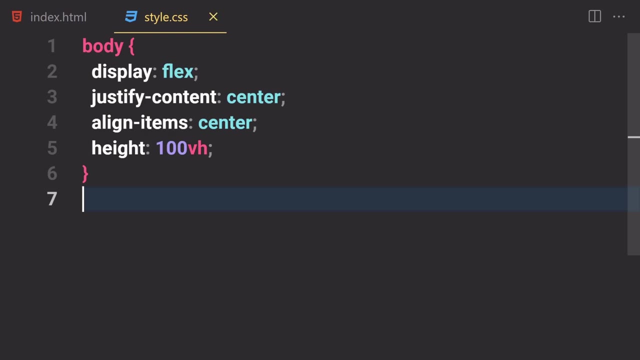 subtraction, multiplication and division. so this is it about a call function. now, the next thing which you have to learn is something called a mix blending mode. so what do we have to do for that? so what i'm going to do is that i'm going to remove this s from here. 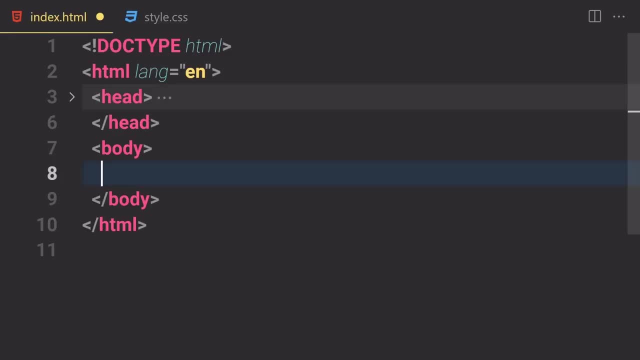 and i'm going to remove this s from here and i'm going to remove this s from here. i'm going to just create a new container right here. so i'm going to create a section with the class of container and inside this section i'm going to just create a div with the class of img. 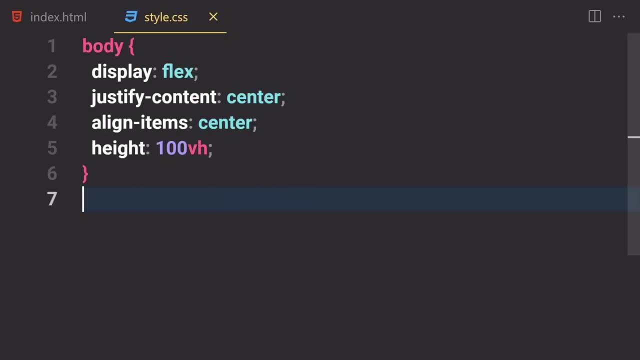 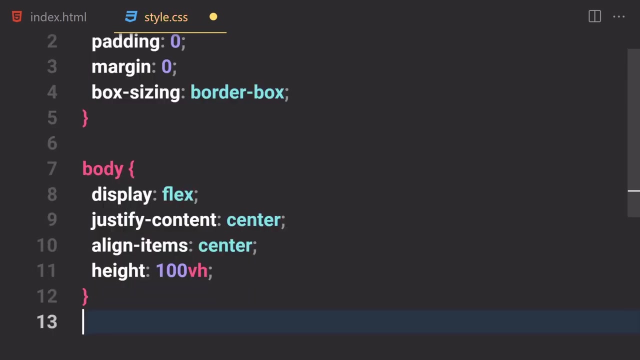 for the image. okay, so now inside a css. what do we have to do inside a css? uh, let's just write our resets first of all, so that we can just get all of their image. so let me just write a padding in here and we can also write a margin, and now let's just use a box. sizing of border box right. 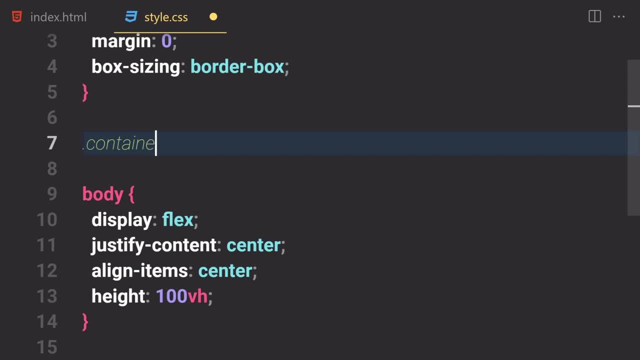 there, okay, so now let's just select our container. so let's just select our container and we have to just use a color of- uh, you know what, instead of color, we can just use a background color of totally red, and i guess that would be fine for. 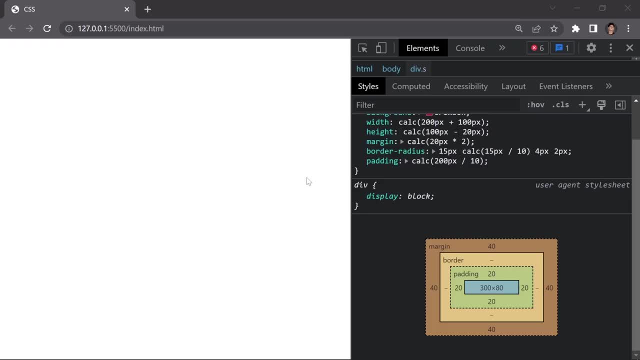 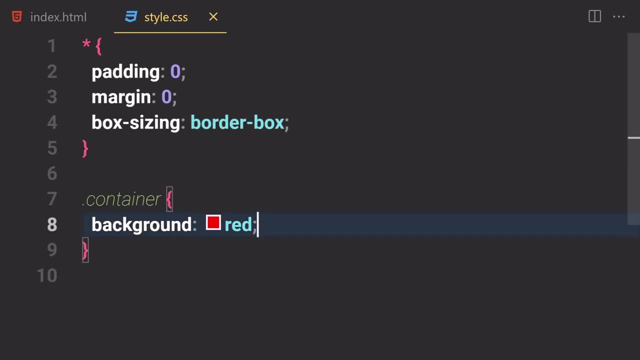 now and i'm going to remove this body from there. so if you save our file and we know that we would get nothing, uh, that's because we don't have any content and padding and stuff like that. so now let's just learn about something called the mix blending mode in css. so the mix blend mode css. 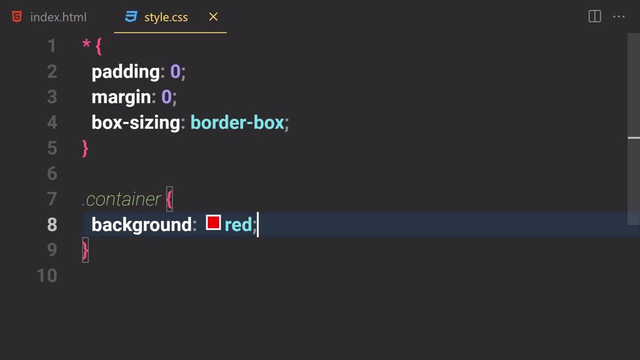 property sets how the elements content should blend with the content of the elements parent and the elements background. okay, so i know that was just quite a crazy terminology and we have a lot of values for that. like we have a normal blend mode, we have multiply, screen overlay, dark and lighten color doors. if you already work with a photoshop, 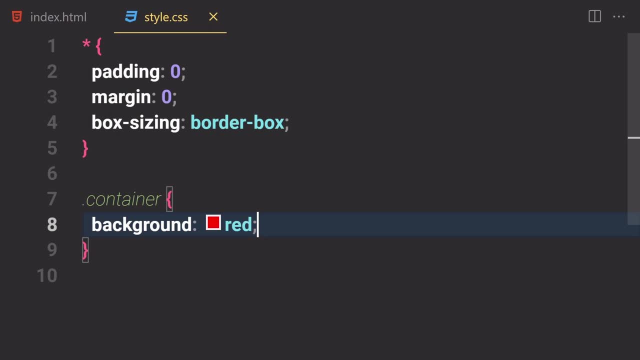 like, if you ever work with a photoshop, so you already know blending mode. so if you haven't worked with photoshop before now, let me just show you what a blending mode is. so now that we select our image right here, so i'm going to go to our image window and select our image from there. 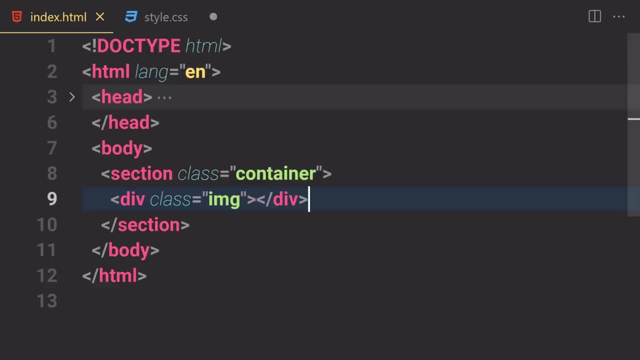 now the next thing which we have to do is that we have to first of all just select our image inside that container, not just an image, but this image div right here. so for that we can just first of all select our container, then our image right here and we provide a class of image, not at all image, right. 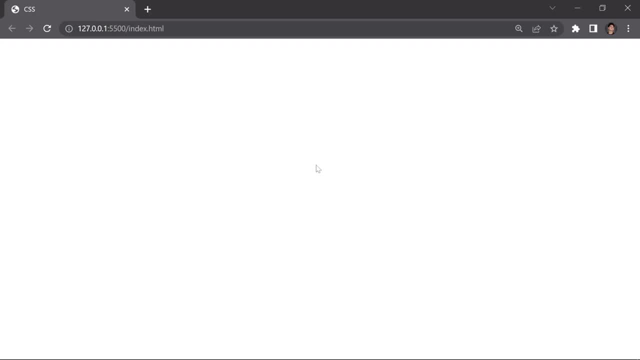 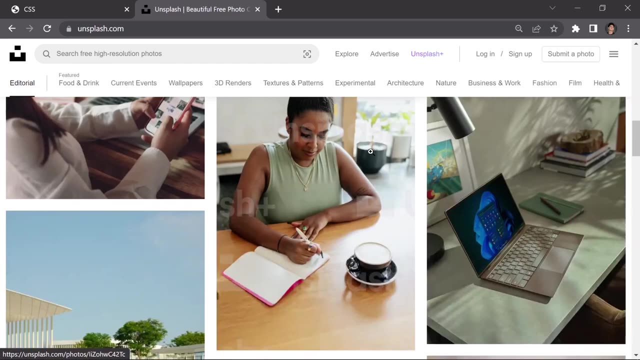 there. so for that we can just use like background image right here and here we have to specify the image path. so now let's just search for image. so i'm going to go to unsplashcom- real quick search, for i don't know which kind of image would be fine, okay, so i'm going to just search for maybe. 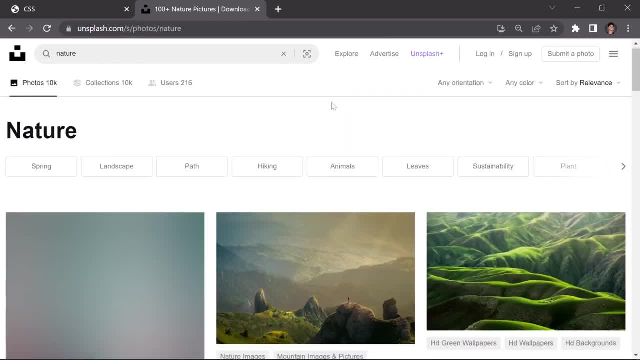 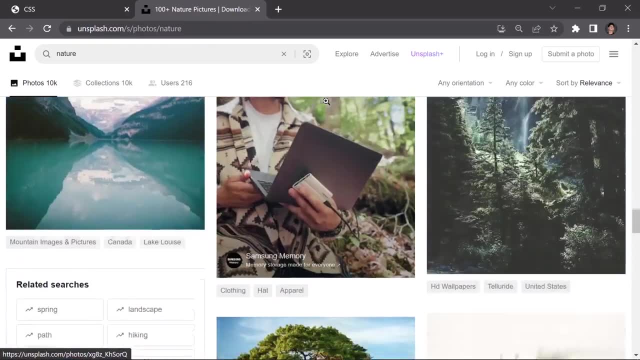 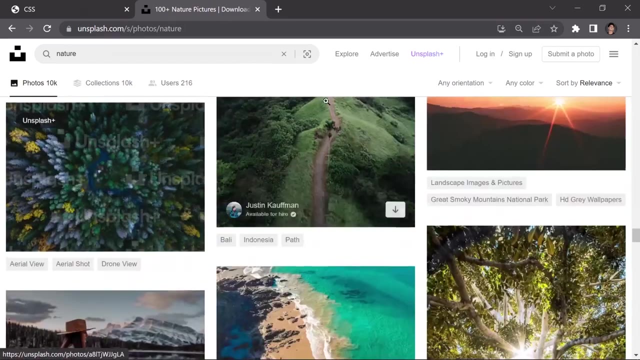 a nature would be fine. so i'm going to just write a nature in here and i guess i'm going to just choose kind of a. um, i don't know which kind of image should i pick. i can pick like whichever kind of image i want, but i want to choose like a cool image for this mix blending mode. so 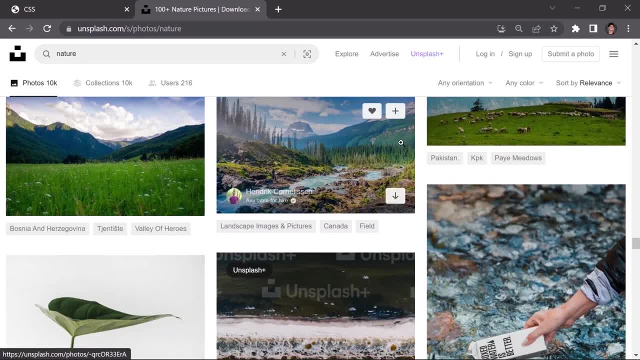 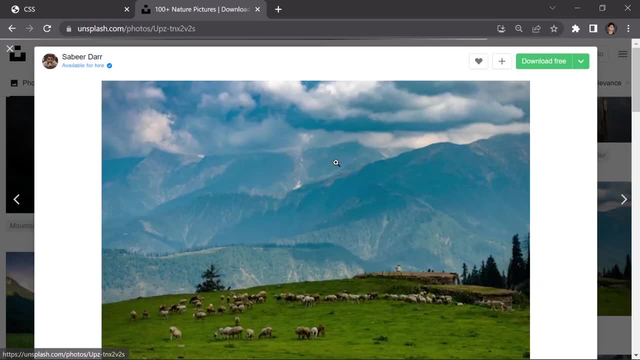 i guess you know all of them are crap. i'm going to just choose this one. we already work on this one once we are working on a filter. so you know i'm going to just click on this image. and now let's just right click on there and copy the image address and i'm going to put this image. 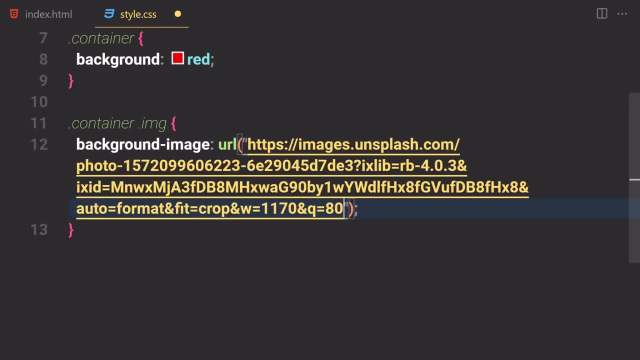 address right here, but inside a quote, so i'm going to zoom out a bit. so this is our image. now let's just use a background repeat of no repeat, because we want our image to do not repeat itself, and background position will be set to center background. 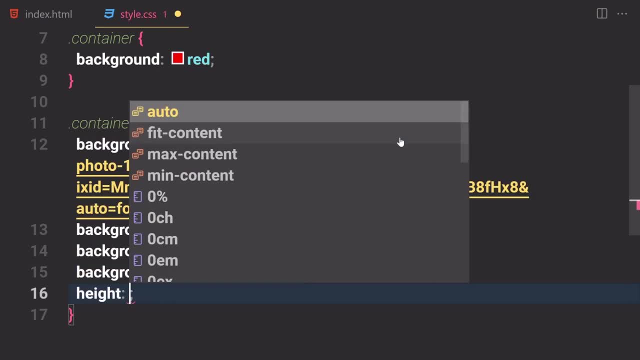 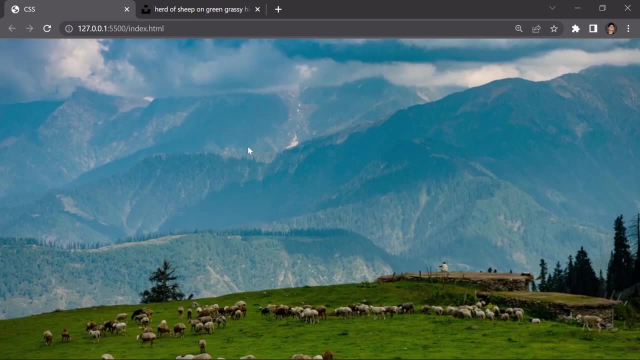 size will be totally covered, okay, so i'm going to also give him a height of 100 vh, so that we can just see everything in 100 vport height. so if you saw that, and now let's just go and here you can see, we are now seeing this image, but it's kind of a crappy image, you know, i'm going to select another. 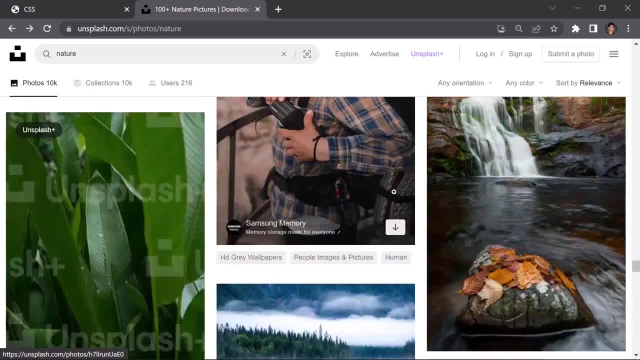 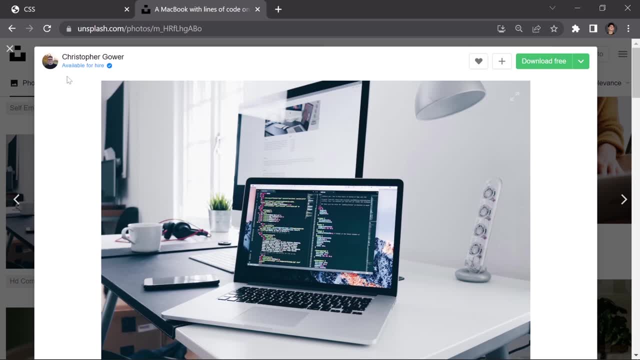 image. you know, this image wasn't the way i expected it to be, so let's just write our computer. you know, i'm going to just select this image from this, uh, i guess. sorry, i can't pronounce his name, but i'm going to just choose this image. 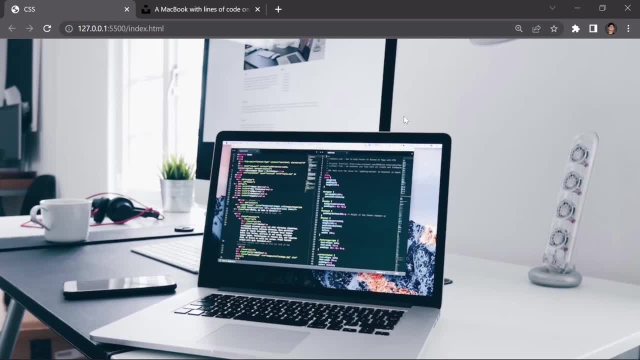 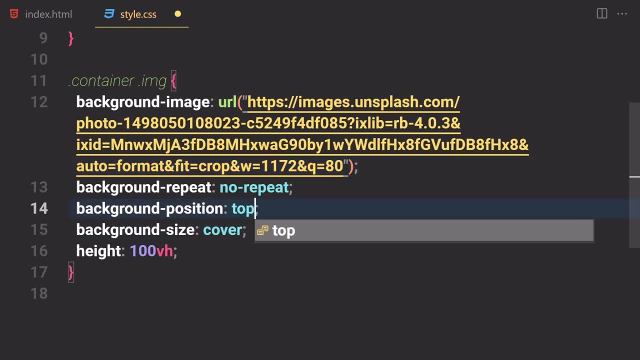 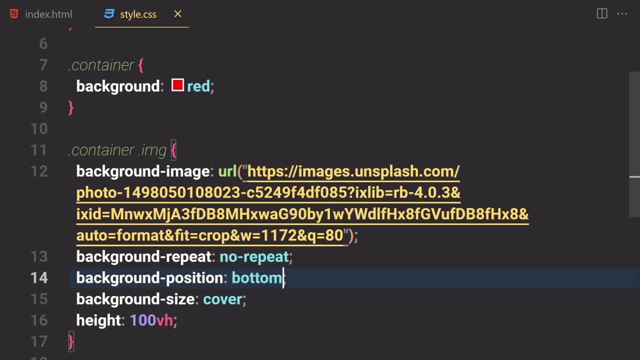 and i'm going to paste it right here. and if you sell that- and i guess we can totally work on this image if you want to, and instead of center i can use top, and if you sell that, it will give us top, but bottom would be fine. yeah, i guess that would be fine. and so now here you can see as the background. 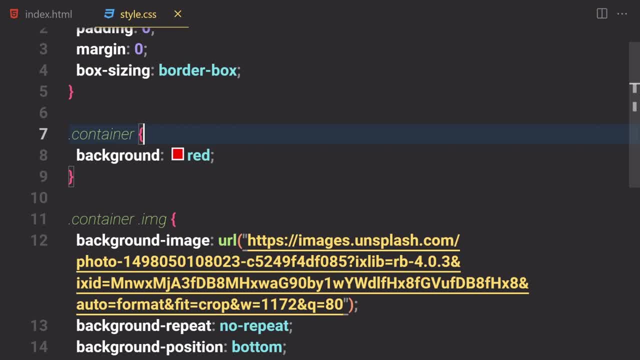 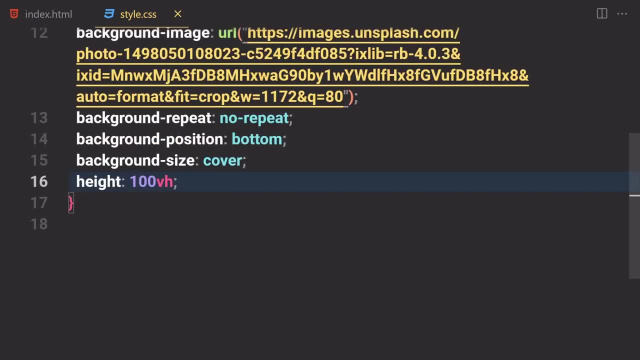 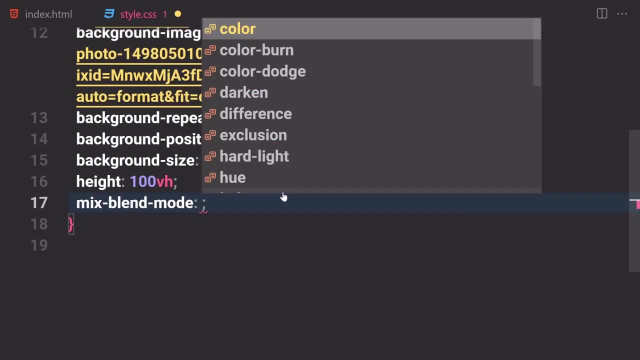 of this container image. we have a red color right here, like we totally set up this um red color as a background right here. and then here we have our image right here. but now let's just use a property called a mix blending mode, so we can just use, like mix blending, our blend mode, to be precise. 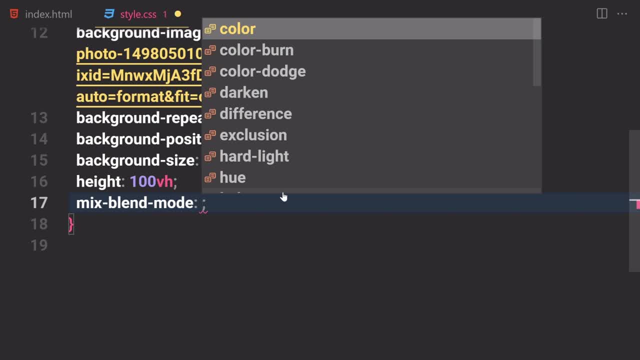 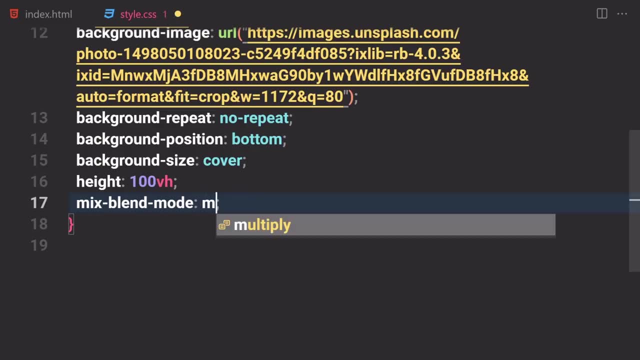 not blending mode, so we can use that. so by default the- i guess the body for- is a normal. so if you save that, nothing will happen right here. so we can also use a multiply. so if you save that, so we'll now just multiply our image and it will now give us kind of a greenish color and we can also change. 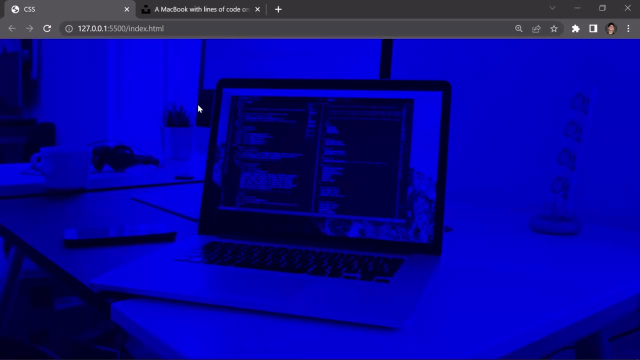 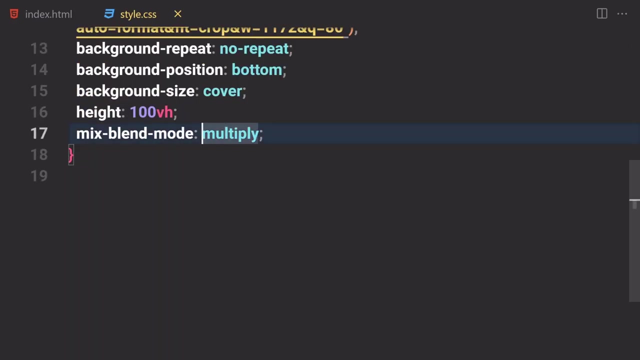 this color to be like blue, if you want to. so if you just use blue, so it will now give us that blue kind of color and then we can just use that blue color to change the color of the image so we can on the foreground. so this is a mix blend mode of multiply we can also use. you know, i'm going. 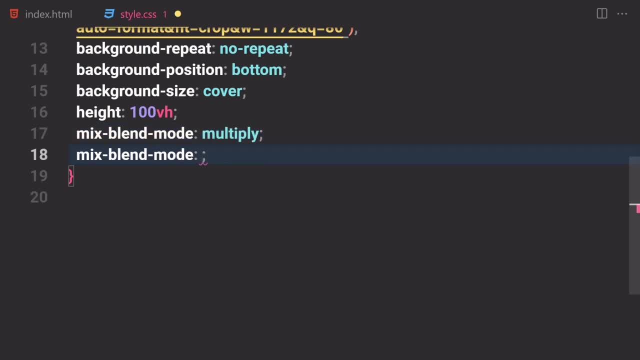 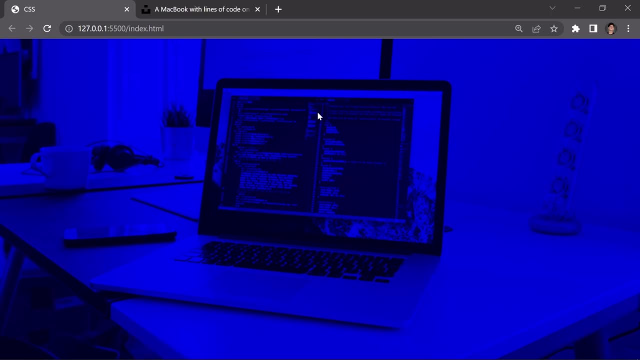 to just duplicate these lines so you guys can see everything in one line, or not in one line, but everything on the screen. so i'm going to just use darken value and if you save that, it will now give us kind of a darken value of that image or that color we can also use. let's just duplicate. 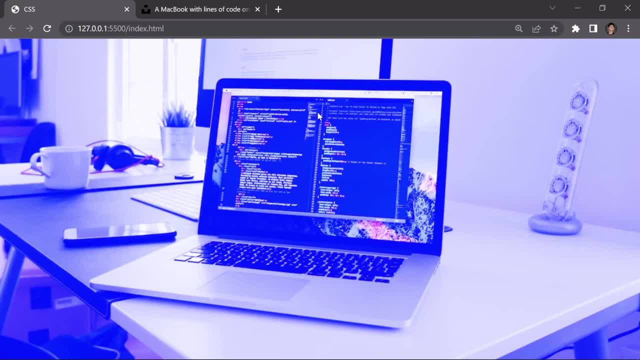 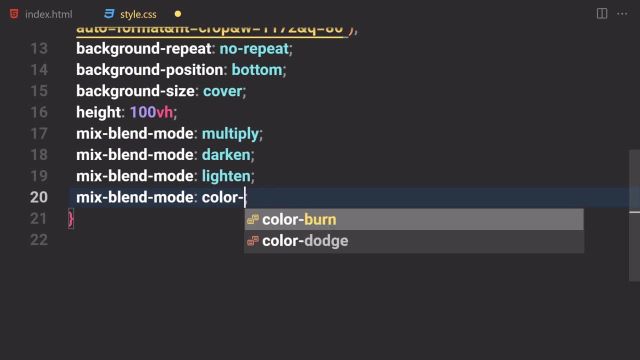 that and we can also use lighten and if you save that and here you can see, it will not use the lighten version of that if you duplicate that and we can play around with that, but i'm going to show you all of these values, so i'm going to just use like color of doji blue and if we save that and it. 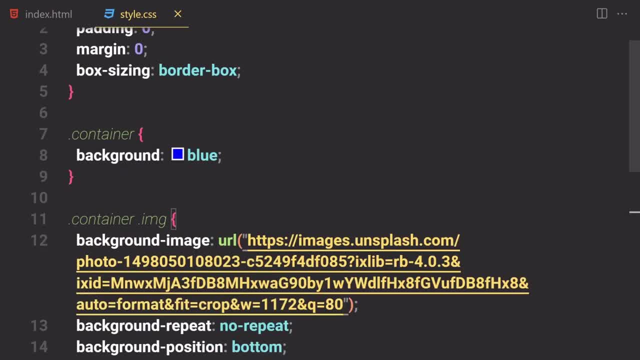 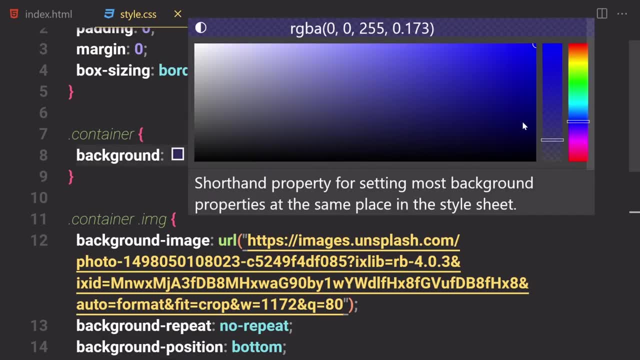 will not just fill out all of the colors, so for that we have to specify some sort of opacity. so i'm going to just decrease its opacity and if you save that, and here you can see, this is how we can play around with this overlay, or what was that color? doji blue or what was that? so we can just 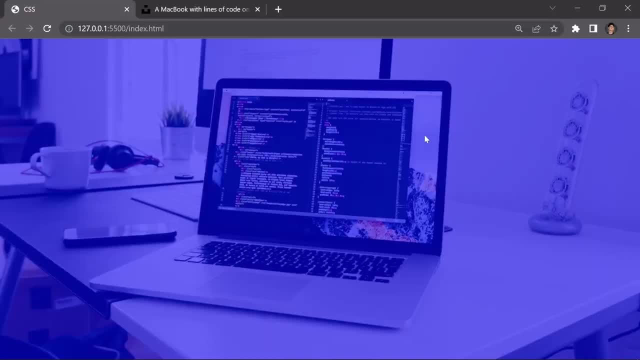 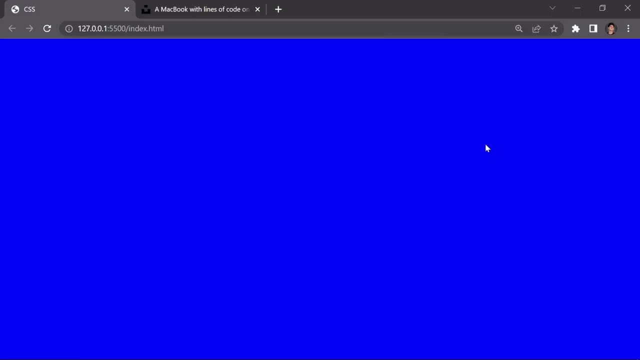 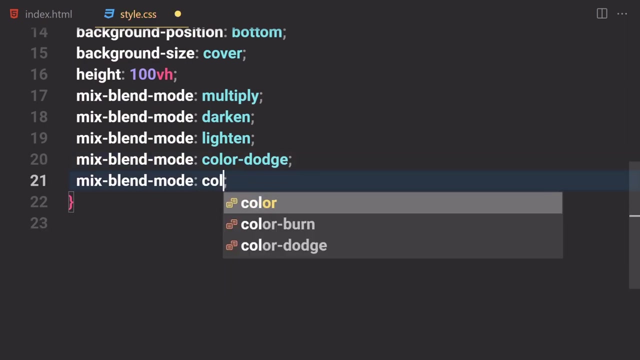 play around with that. so if you get like only pure color, like this one, if you just specify instead of providing a, instead of providing opacity, so if you just get like totally blue color, so for that we have to change the opacity of that color, so now let's just duplicate that, now let's just provide a color, burn or burn whatever. however, 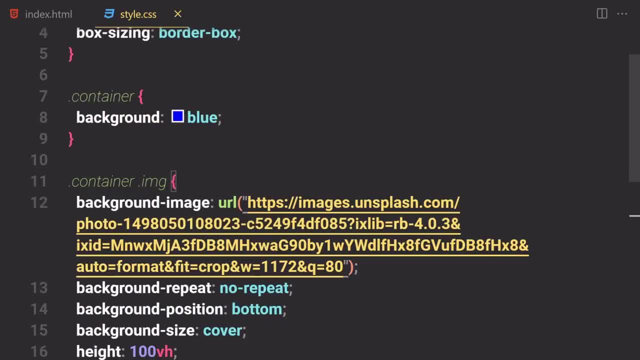 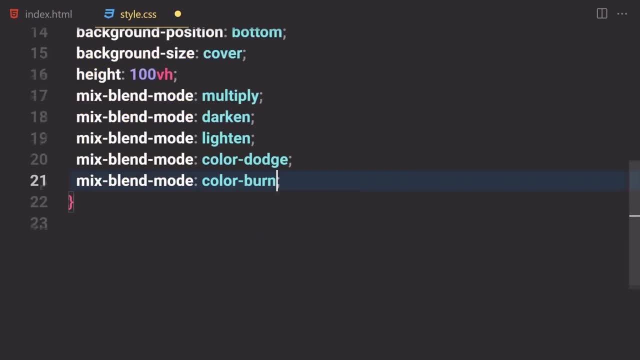 you want to pronounce that and if you save that, okay, so it's still giving us that kind of a image, or so now let's just change the opacity, and here you can see this- how we can play around with that, so duplicate it now. the next value which you're going to be using is our differences, or difference would be fine, and 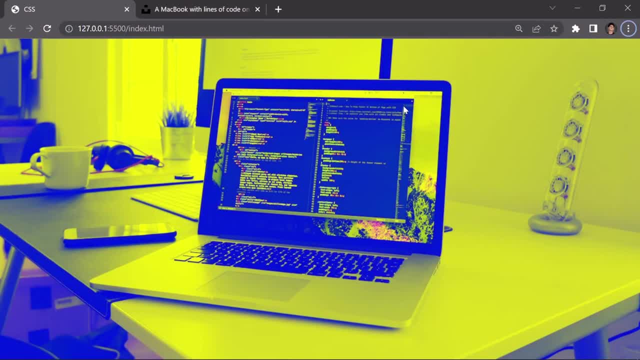 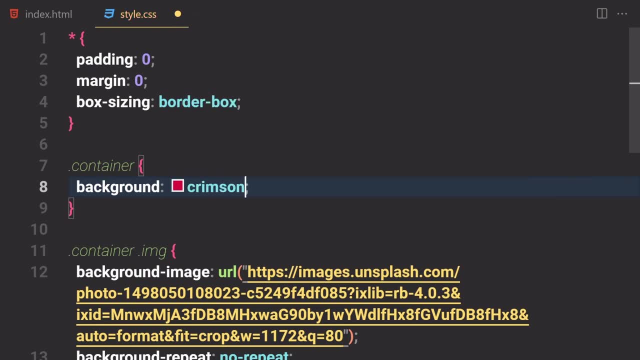 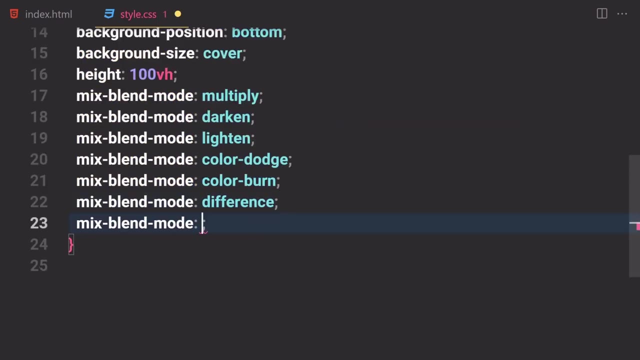 if you save that and fill log uses a difference based on that image and that color. so if you change this color to maybe like uh, sky blue or not, sky blue like crimson- and if you save that, certain log uses the differences between the color and the image. now let's just duplicate that and 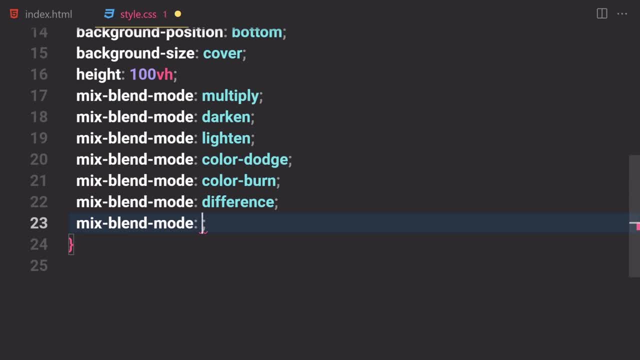 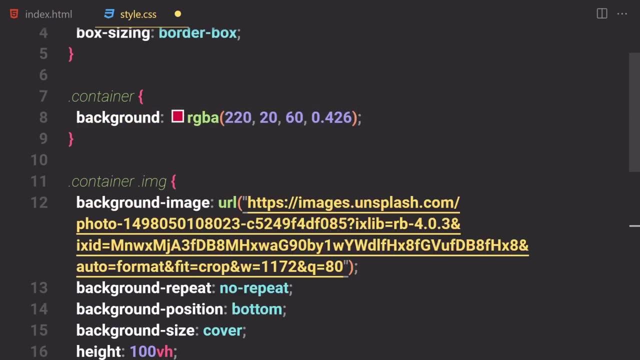 you can just play around with that if you want to. and now let's just use another property. and now, if you save that- and here you can see these subtle differences- now let's use a hue one, so save it. it will not use a pure hue. we can decrease the opacity if you want to, just like that. 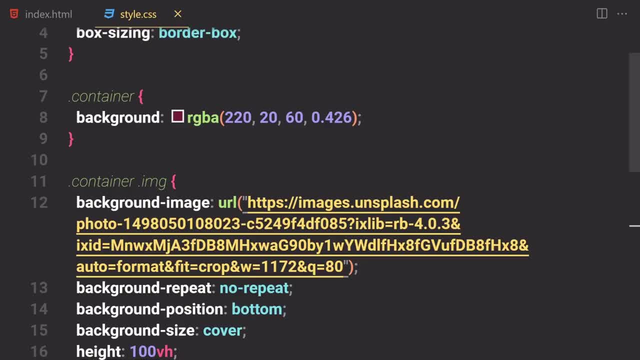 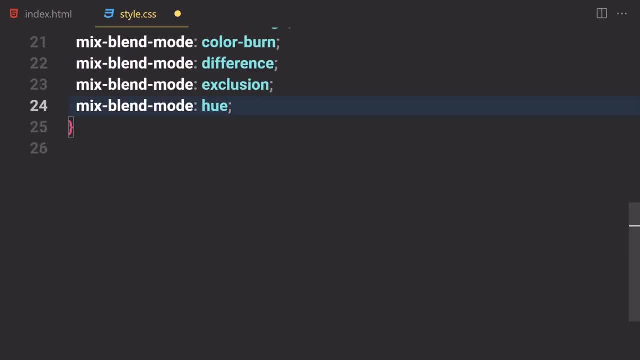 and i'm going to save my file and this is how we can decrease the opacity. so if you decrease the opacity, so we will get a lot of different kind of results. so i don't want to decrease the opacity, so you would be fine. now we can use a saturation if you want to. so i'm going. 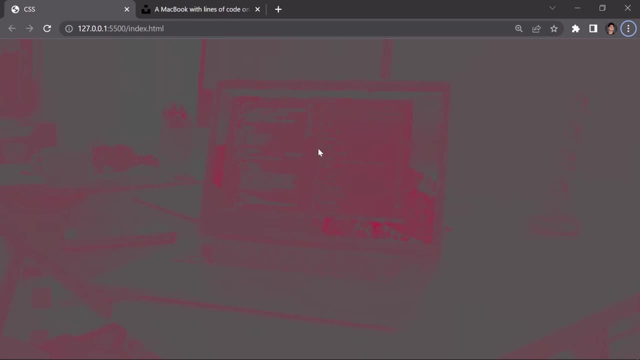 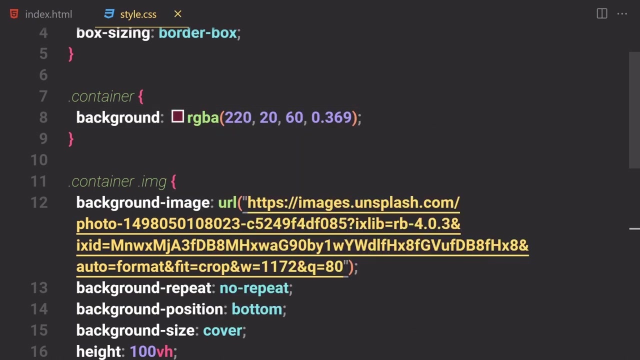 to just provide a saturation and if you save that, it will not give this pure saturation right here, so we can just decrease the opacity and we can play around with this color. so if you save that, so it will now give us a little bit saturation and we already learned about saturation on our 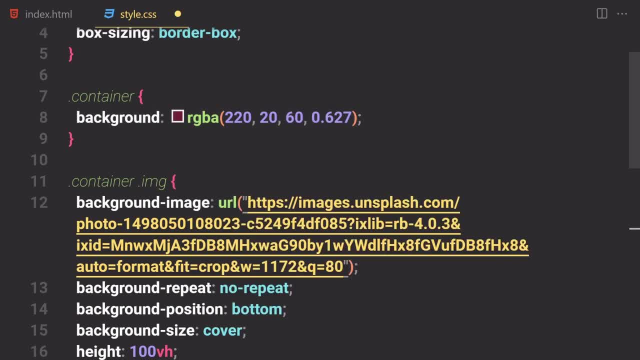 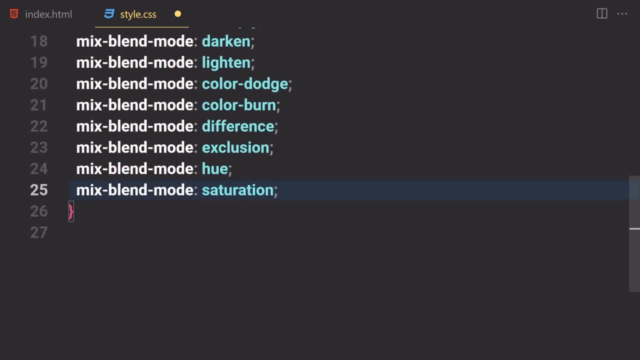 filters and gradients for you, if you remember that. so we can use saturation there and we can also use it here if you want to. so now let's just change everything to pure color and we can also provide a color right here. so if you just provide color and if you save that, and it will give us. 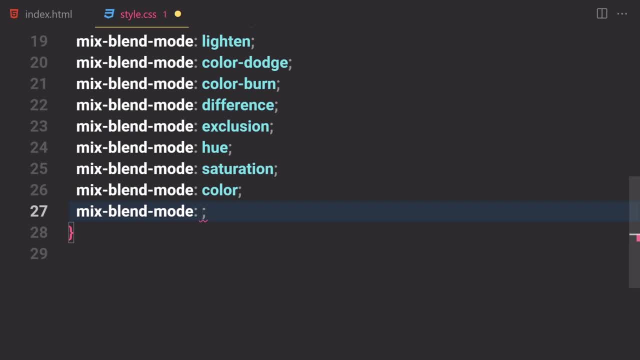 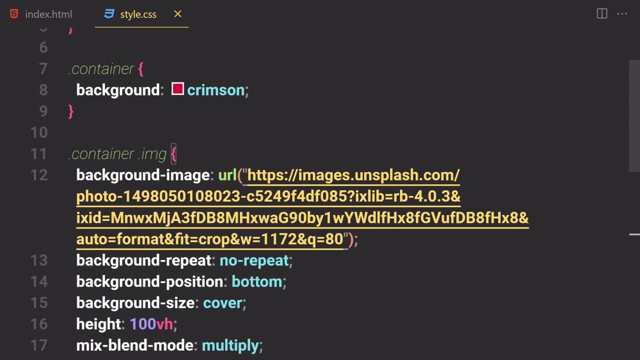 result based on that. and now let's just write a loss property which is like: sorry, i can't pronounce this name, but luminosity- yeah, i can't pronounce the luminosity- and if you save that and here you can see, it will now give us different kind of result based on this color. so if you change that, 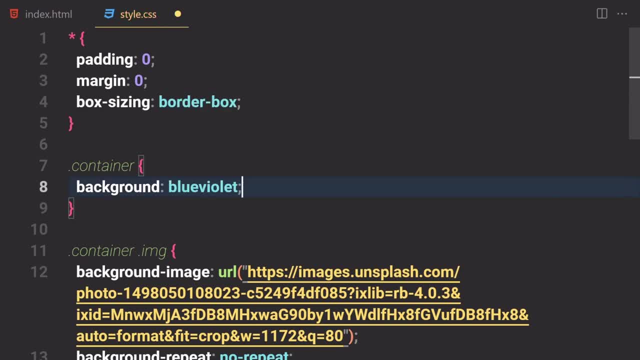 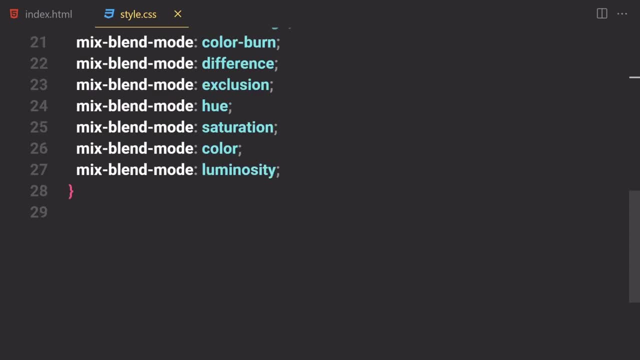 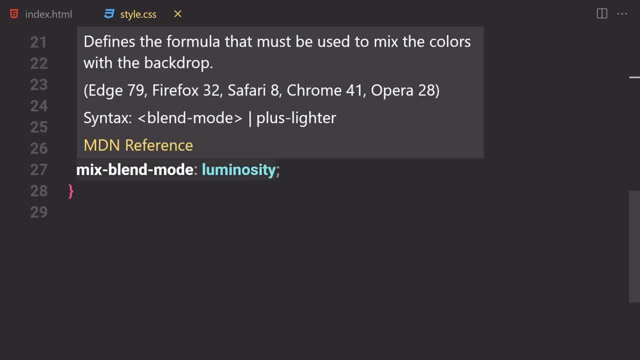 okay. so now let's just, uh, use it a little bit more, and then you'll get to know what is the usage of this mix blend mode. you, uh, we can also use that with gradients, if you want to. so, uh, you know what. i'm going to remove all of this mix blend mode from there. and now the next thing which you 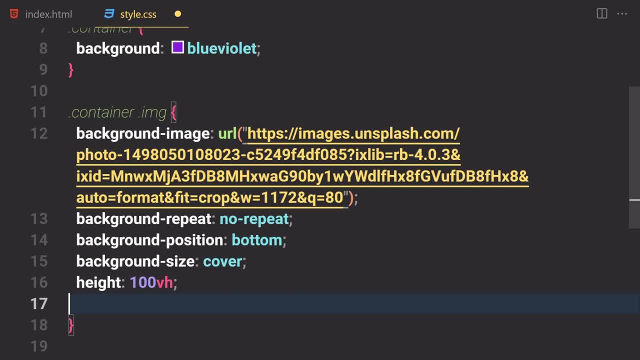 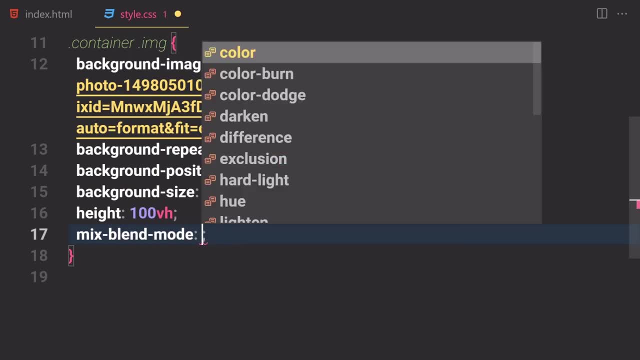 have to do is that here we have to specify the linear gradient. so at the end of this image, first of all let me just try to mix uh blend mode and we can now use, uh, maybe, the overlay one. so now let's just do that and we can now use the gradient mode. and we can now use the gradient mode and we 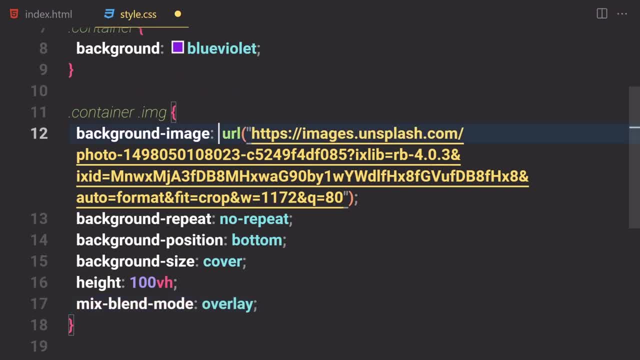 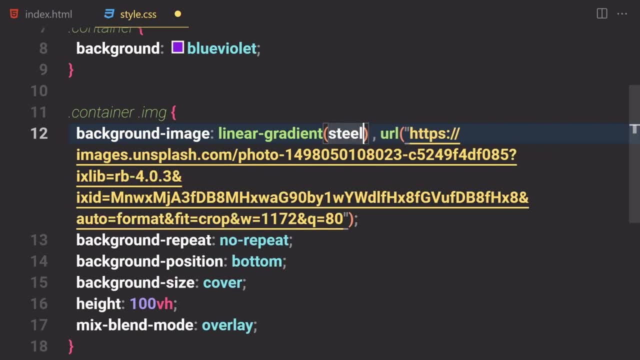 let's just use the overlay and we can also use the linear gradients if you want to. okay, so let's just use a linear and gradient, and here we are going to be specifying like a steel blue color and also, uh, that fire brick color. so i'm going to just write a fire brick. so if you save that, 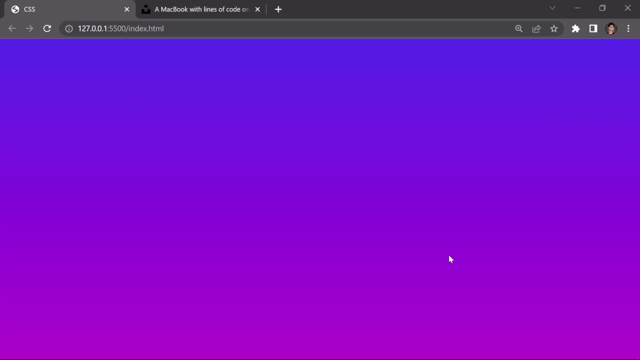 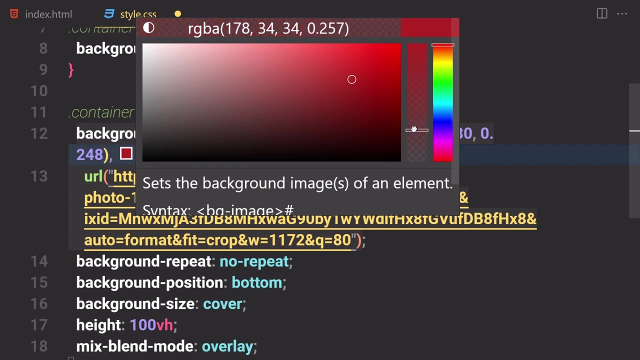 or fabric, however you want to pronounce- that if you save that, it will give us kind of a gradient right here, but we have to change its opacity as well, so we can just decrease its opacity and we can play around with that. so if you save that and it will give us results based on that, okay, so here you can see our mix. 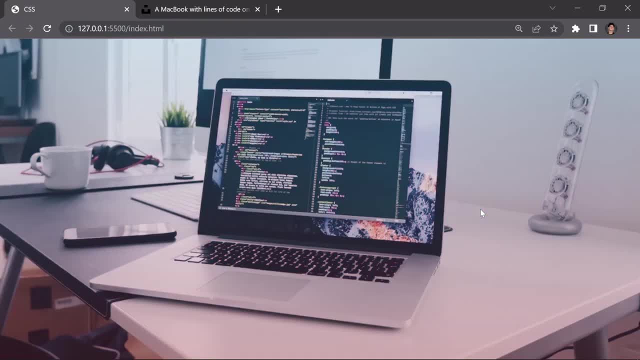 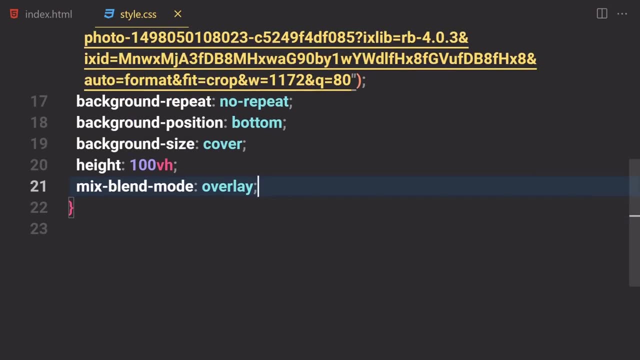 blend mode is set to overlay and if you comment this line out and if you save that, so this is how our gradient will look like if you uncomment it and save it, and this is how we can use a mix uh blend mode on that we can use like, maybe a different kind of value, like, maybe, i don't know. 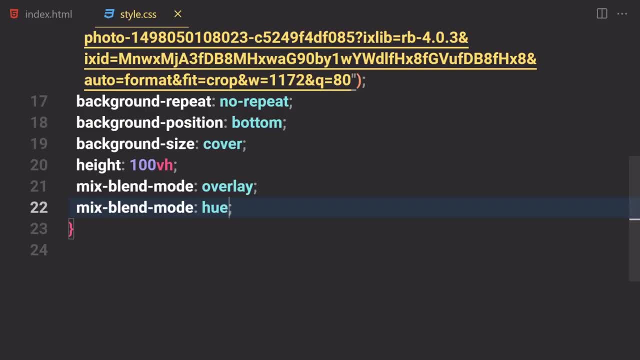 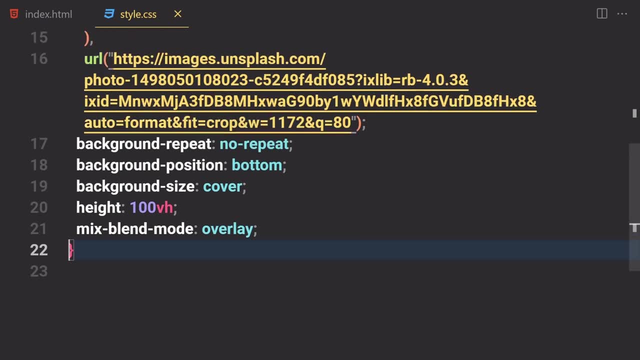 if you use hue, so we're not going to use a result based on that hue, and i already show you all of these values so you can play around with that in your free time if you want to- and, by the way, i'm going to come back to this product. i'm going to tell you what we're going to do here. okay, we're. 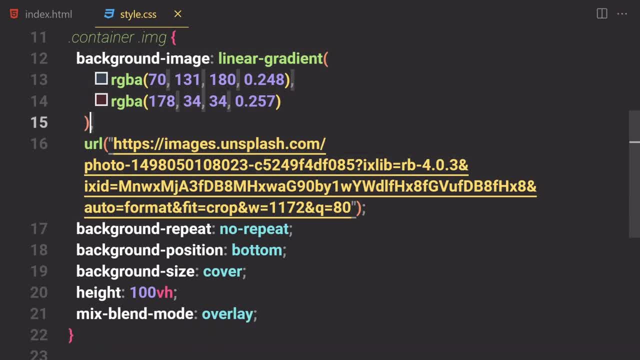 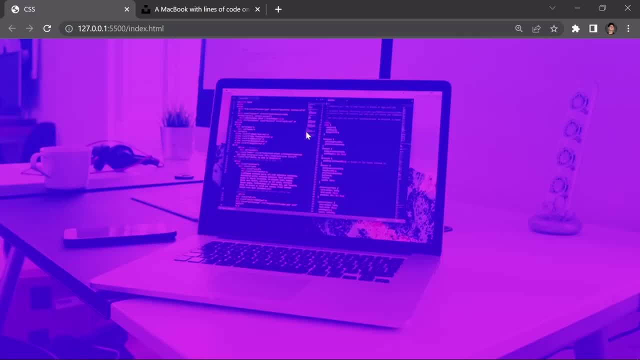 going to need to do something different. okay, so let's just get another image of, maybe, a macbook or whatever we have. so i'm going to just select this image, maybe. or i guess i'm going to select this image and now i'm going to right click on that and copy the image address. and what do we? 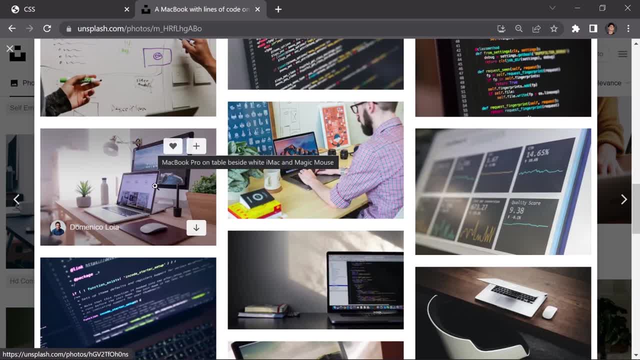 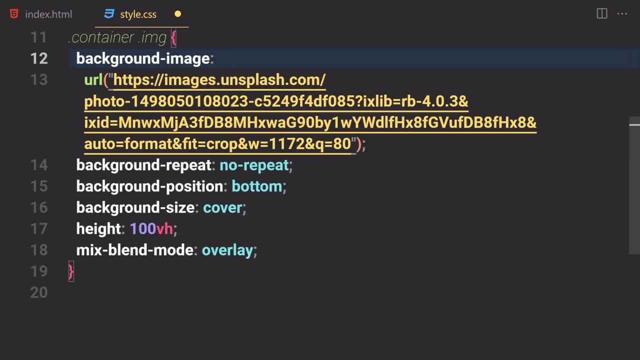 have to do. i'm going to first of all put a comma in there, and then i'm going to put a comma again, and then i'm going to paste in the name of the image and then i'm going to move this to the image and i'm going to type in the name of my image here. 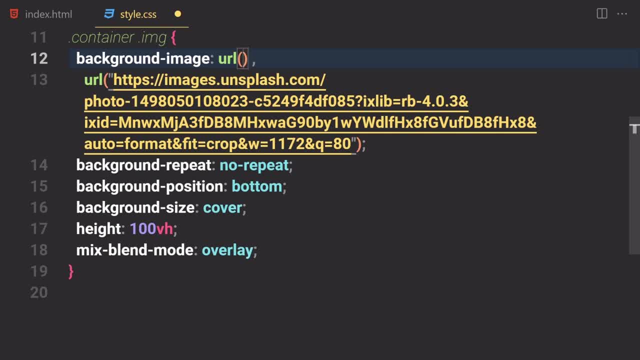 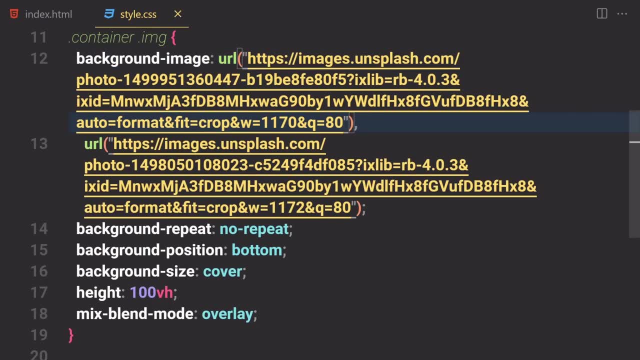 and now here i'm going to just write like a url, so this will be the first image and this one will be the second one. so i'm going to just put its image value so, or link, so, if you save that and if you check it out. so here you can see, we are now getting this one image, but we cannot see the. 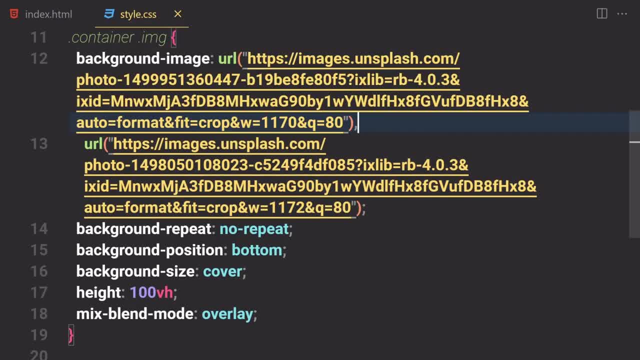 other one. uh, so now let's just play around with there real quick, but then we can just use a linear gradient as well. so let's just put a comma in there and i'm going to put that linear gradient in here and i'm going to pour like a steel blue color, and we can also pour like a fire brick color. 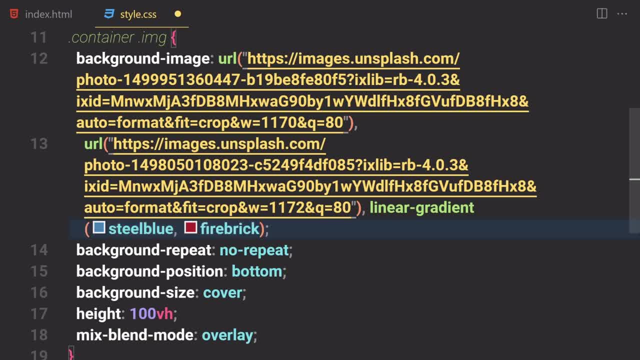 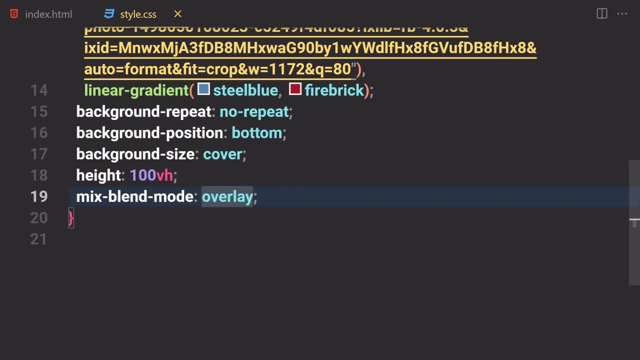 as well, and let's just change its opacity from somewhere else. and now if you save a file, and this is how this image looks like, but we cannot see that other image, so for that let's just use like multiply and also comma screen, and if you save that, uh, okay, so we are getting a totally 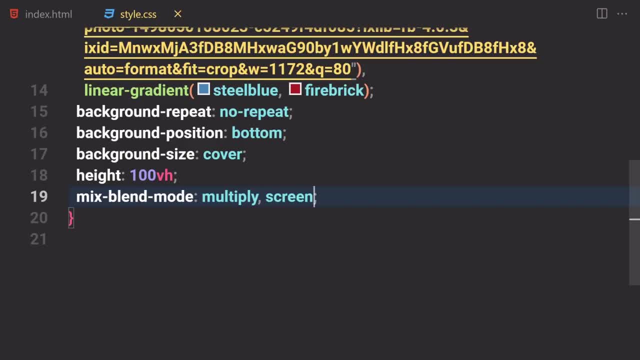 different result. i guess something is wrong. so instead of using a mix blending mode, we can use, uh, a background blend mode. so if you just use like background blend mode and if you save that and here you can see, we are now getting these two images. so here you can see. this is the first image. 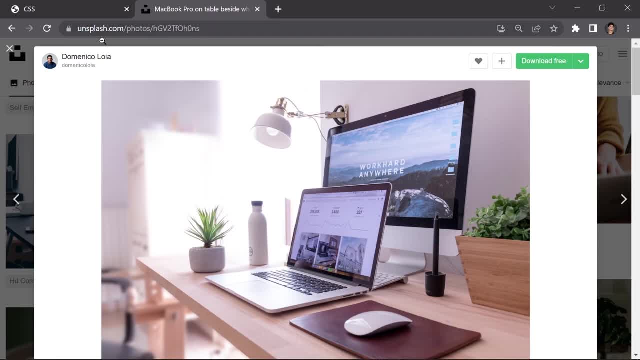 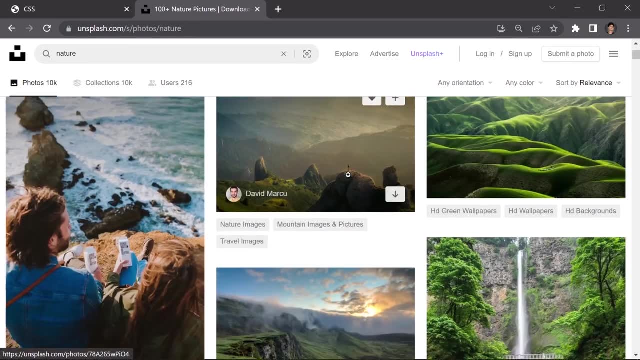 and this one is the second image. we are now seeing that, but these images are crap as hell, so we have to search for another image. so i'm going to search for nature and now let's just get like two images. i'm going to just click on this one and then right click on that and copy. 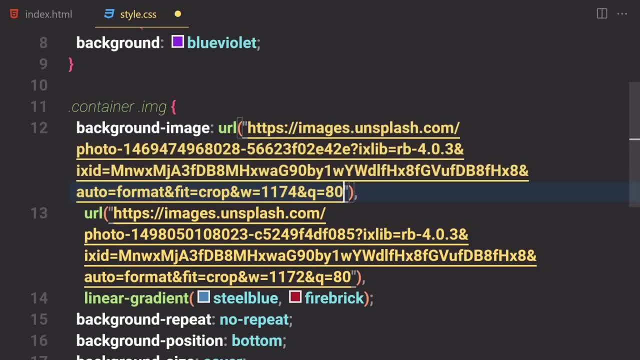 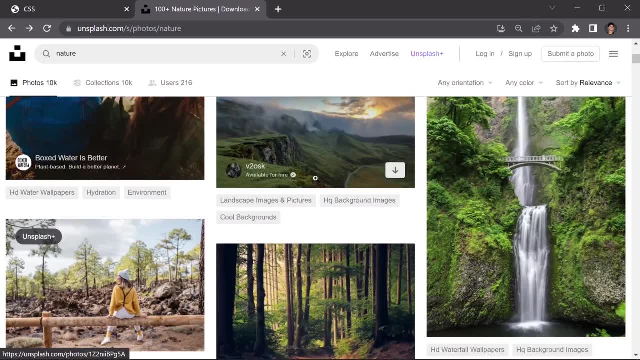 the image address and i'm going to put it at the first image, right here and now let's just search for another image. maybe, like i don't know which kind of image would be fine, i'm going to search for, or, you know, i'm going to click on this image and now let's just right click on it and copy the. 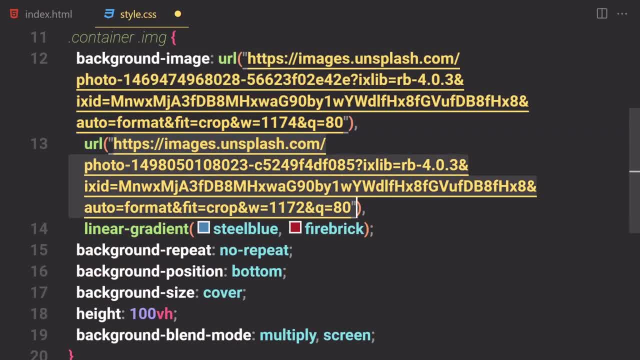 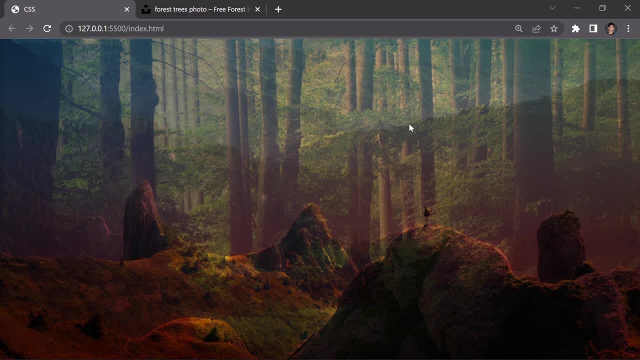 image address and i'm going to put this image address in the second area right here and now. if you save that, and here you can see, we are now getting two images, two kind of different images. so this is our three images. uh, so here you can see, these are our three images and this is a. 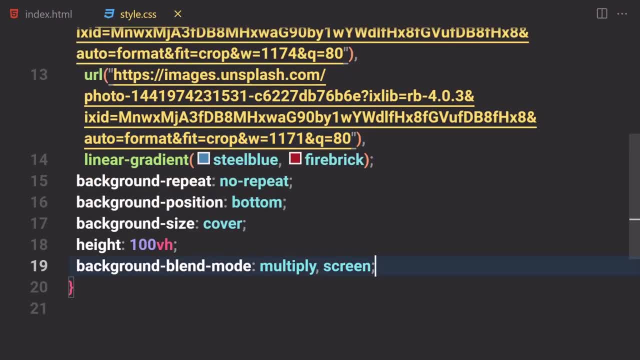 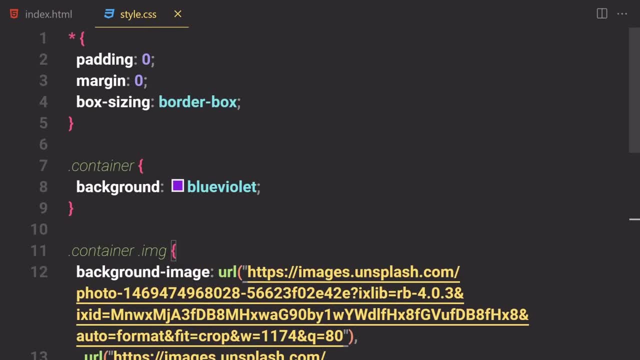 mountain image. so this is how we can play around with a background, uh, background blend mode, and this is how we can play around with the mix blend mode in css. so, now that we are totally done with the mix blending mode and background blend mode, so now the next thing which we have to learn is 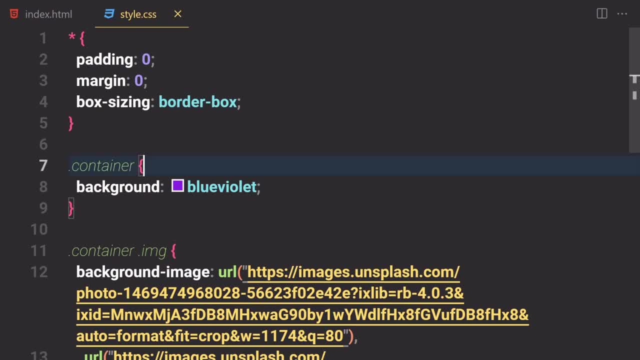 something called a is pseudo selector. we already learned a few pseudo selector back when we were learning about like howard visited and that kind of pseudo selectors. so now in this video, or now in this section to be precise, we are going to be using uh is pseudo selector. so we are going to be. 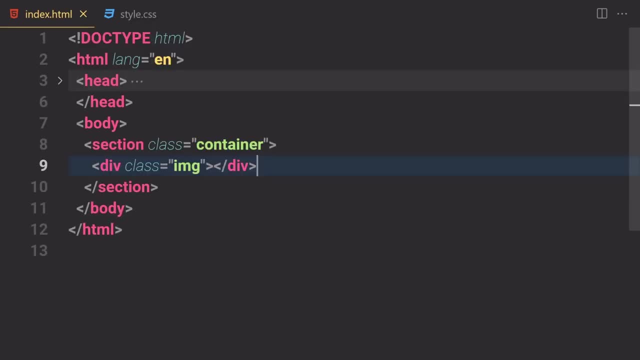 using is pseudo selector, so we are going to be using: uh is pseudo selector, so i'm going to just remove everything from here, and now let's just get into our html and now let's just remove this section and stuff. so for that we first of all have to write a header and inside this header, 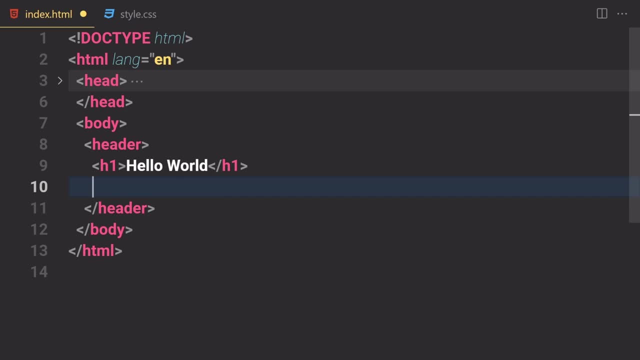 we just have to write h1 of like hello world, and then, you know, i'm going to just put like hello, word of one in here, and now let's just use h2 of hello, word of two, and now let's just use h3 of hello word, and then three. okay, so now we are totally done with the html. 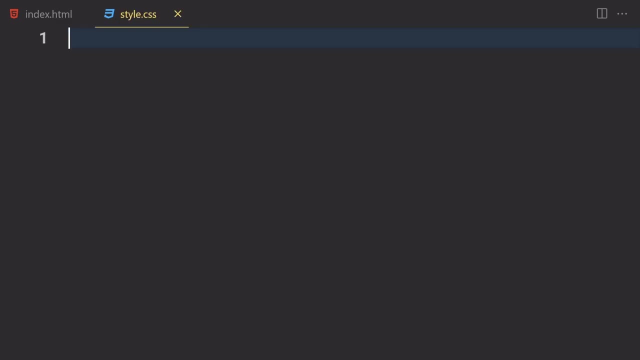 side. now let's just save there. and now inside a css. now let's just discuss about that property called the is pseudo selector. okay, first of all, we have to put a column in there, so the css is pseudo selector or the is class, or however you want to call. that takes a selector list like this: 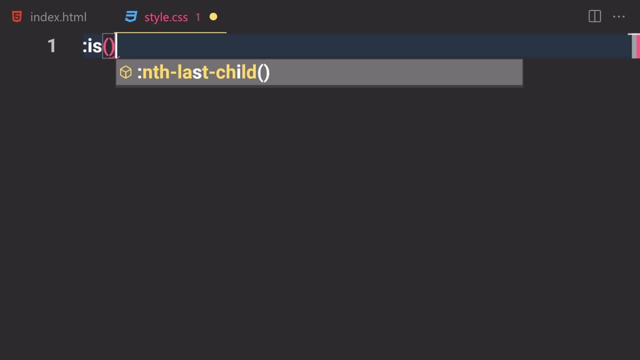 pseudo selector takes a selector list as an argument and select any element that can be selected by one of the selector in that list. okay, so i know this is kind of a gibberish, but now let me just write some code, then you will get to know what i'm talking about. so if you want to select, 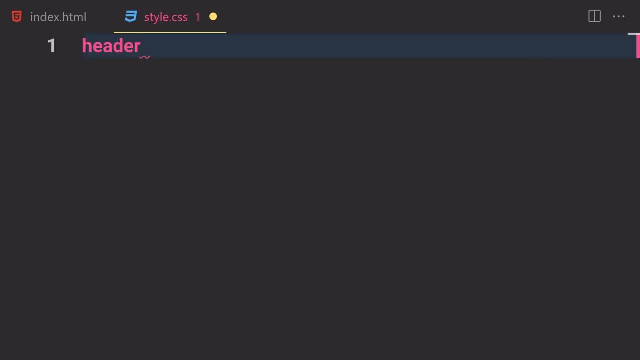 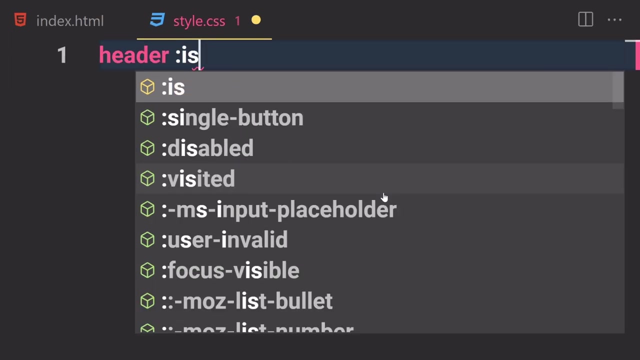 that header. first of all, we just have to write a header and now let's just use that pseudo selector. so we are going to be using a colon. let me just zoom in a bit. we are going to be using a colon and then the is operator or word, however you want to call that, and here we are going to be passing. 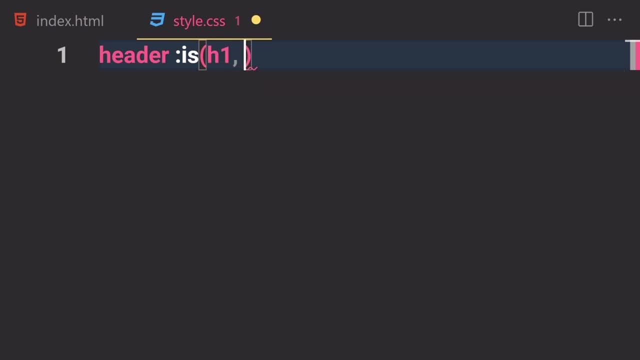 the list of the selector. so we are going to be using like: h1, h2, comma, h3. okay, so we are selecting these three elements inside this header for now. okay, so now inside there, let's suppose if you want to change the color of them to be like: 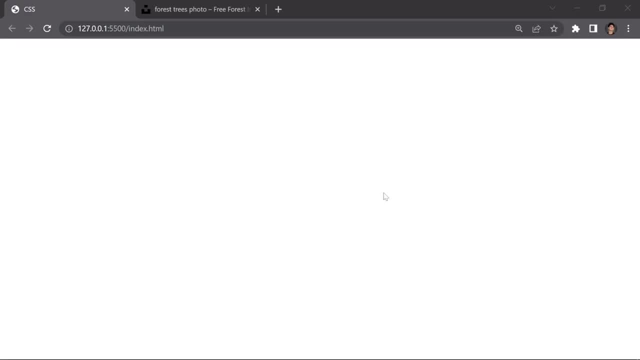 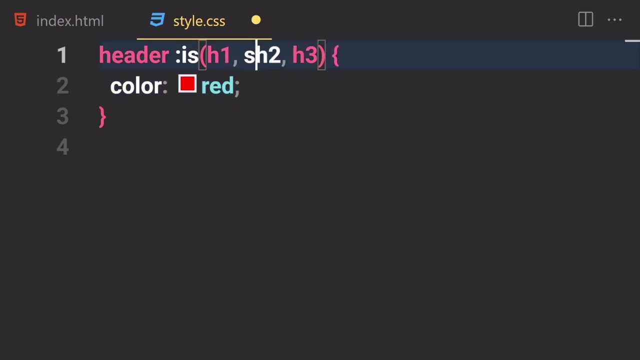 maybe red. so if you want to provide red color and if you save that and here you can see all of them are now totally red. so in some cases we would get error, like, let's suppose if i just put s in there and if you save our file, so it will not just select both of these two and it will not select. 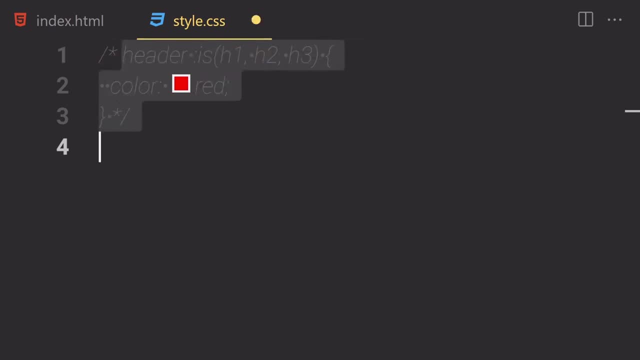 this one. so now, that was just a first example, so i'm going to comment that, or, you know, i'm going to delete that for now and i'm going to also delete this header area from here. that was just a basic syntax, so i'm going to just write a crazy html for now and you have to type it with me as well. 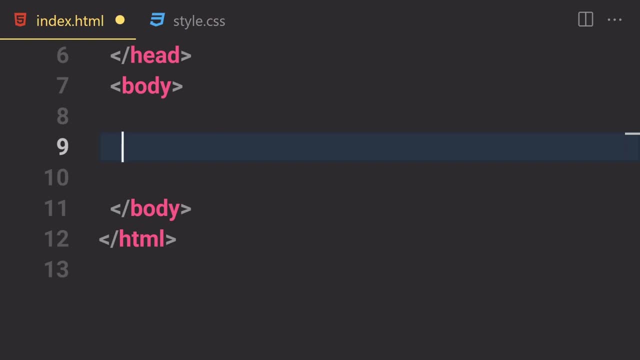 so for now, we are going to be using a section- let me just write a section- with no classes and nothing inside there. uh, nothing, not nothing. but we are not going to be providing any clauses and ids, so we are going to be using h1 of, like uh, section heading one, and now let's just duplicate that a. 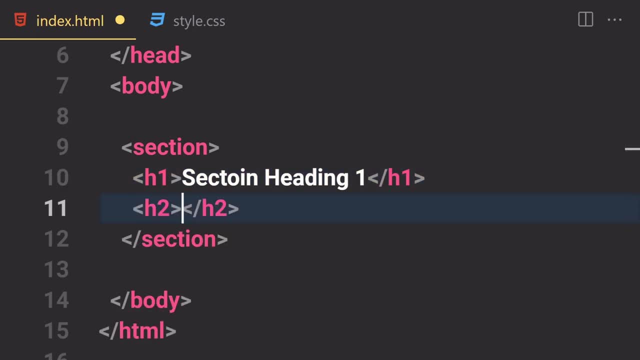 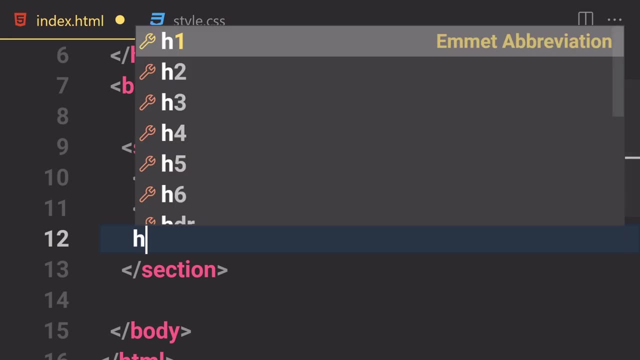 few times: uh. you know what, instead of duplicating that, we are going to be writing in manually like uh, h3, and then we have to substitute that h3. okay, and that's what you're going to be using now. we're going to be writing h3 and section uh, section heading two. now let's just use h3. 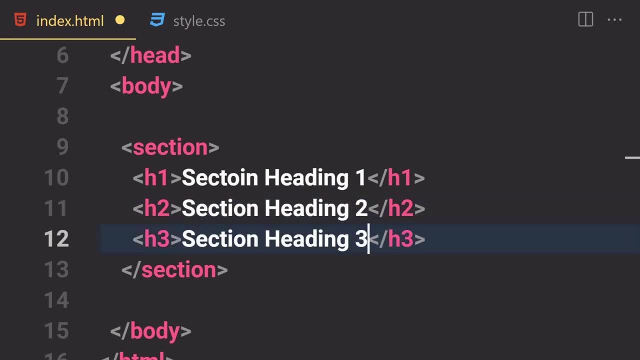 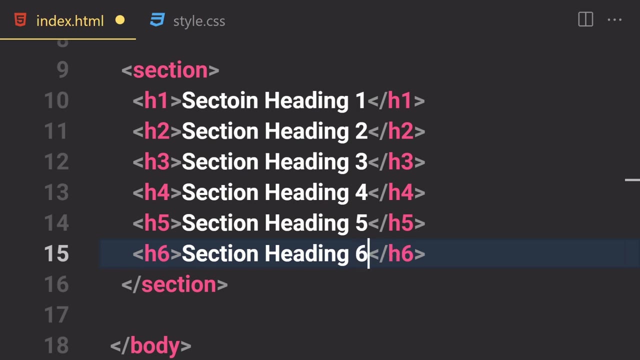 and here we are going to be using a section, or you know, i'm going to copy and paste it. so copy it and paste it, and this one will be now the third one. now let's just use h4 and section heading four. now let's just put h5 of section heading five and finally we are going to be writing, uh, at six for a. 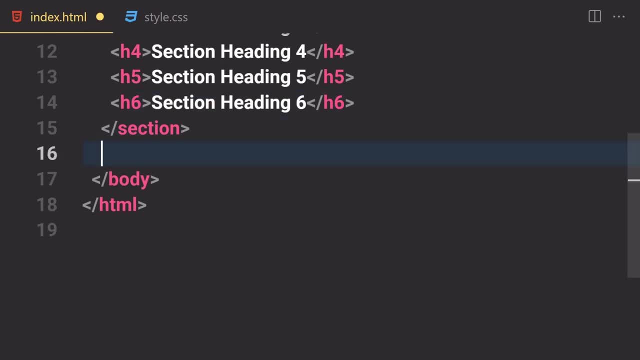 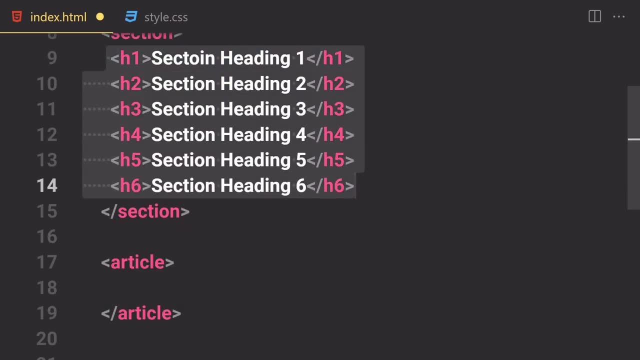 to be the first section. now, the next thing which we have to do is that here we are going to be using articles, so i'm going to just write article in there, and what do we have to do? i'm going to copy all of the content from here and i'm going to paste it right here and now. i'm going to just 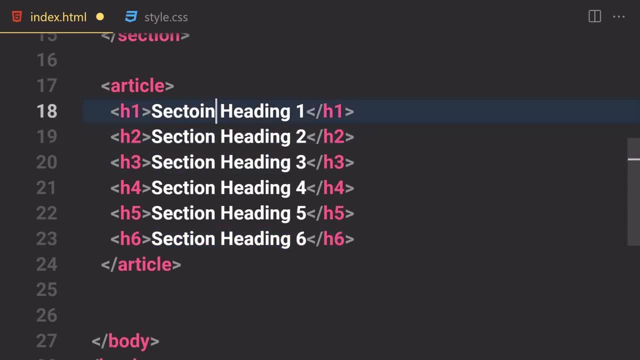 select my section and like so. now, if you want to do multiple selections, so first of all you just have to hold alt and then you just have to click on the selection where you want to make. so i'm going to just remove there and i'm going to put that like article in here. okay, so now let's just 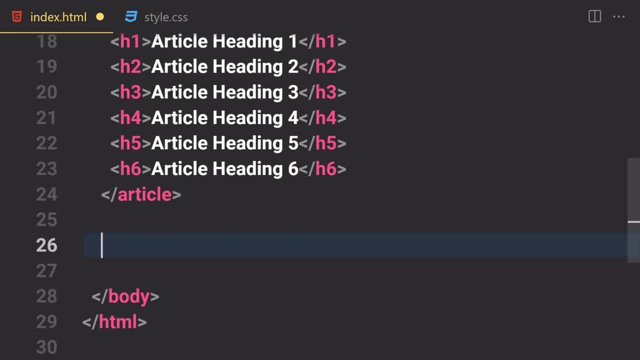 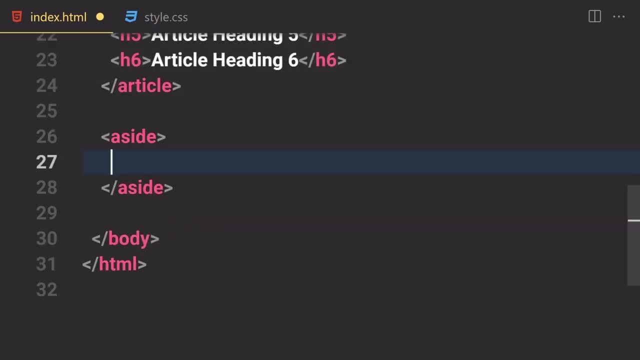 duplicate this section as well, or you know what not going to be duplicating there? we are going to be using a side, so use a sign. and now let's just copy all of this content and i'm going to do multiple selections in here. let's just do a multiple selection in here, real quick. 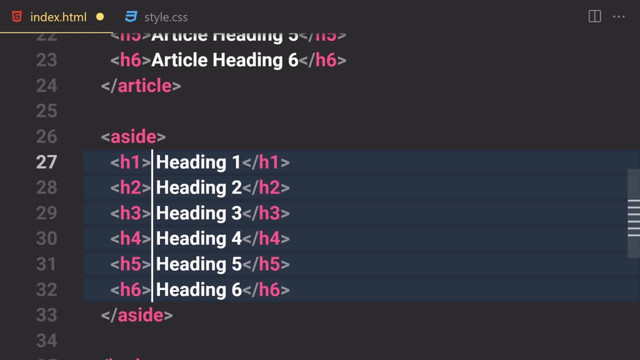 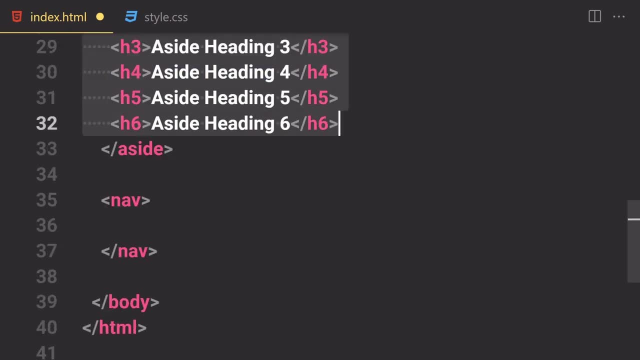 okay, so we messed up in there. let's just remove the other one, and here we are going to be using a site. and finally, we are going to be creating a nav tag, and now let's just copy all of its content, and i'm going to paste it right here. and now let's. 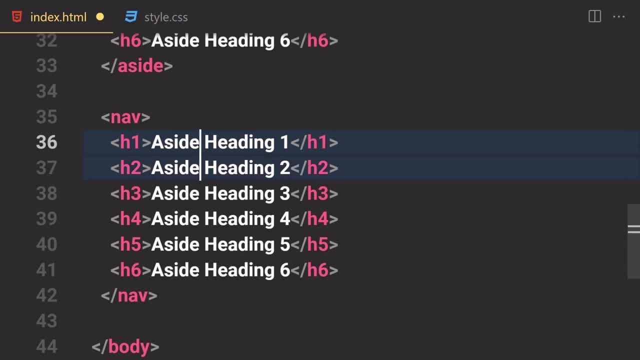 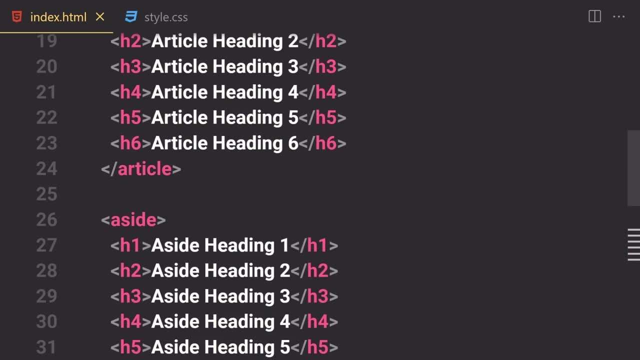 just change this aside to: uh, let's just do a multiple selection, and now let's just change that real quick to a nav, heading one and heading two, and so on and so forth. so this is how currently things looks like. so we have a section headings, then we have article headings, then we have our 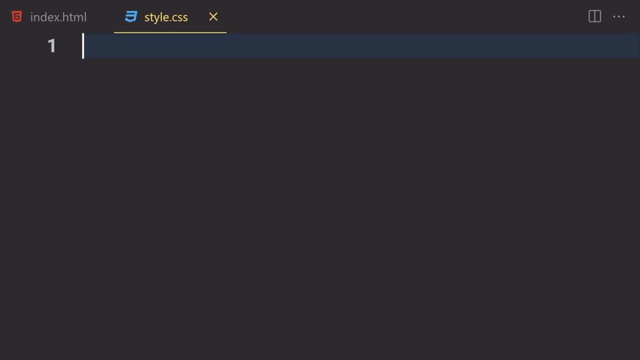 sign headings and then we have a navigation headings. so if you want to select everything, so for that we can just write a crazy amount of selection. so we can just write like section of h1 and then write, uh, section h2, then write a section- you know i'm going to duplicate that- a. 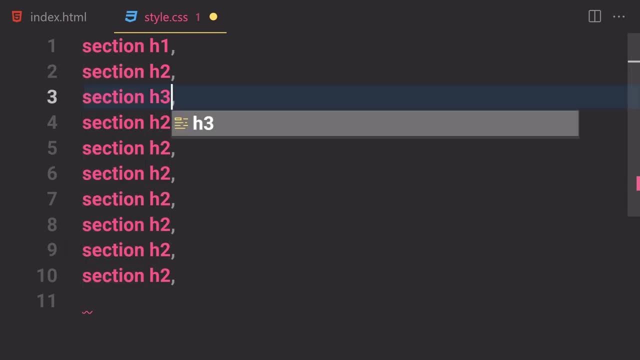 few times like so, and we are going to be writing like h3, h4 of section 5, 6, and then we have to use all of that. so i'm going to just do a multiple selection in there and here i'm going to just use: 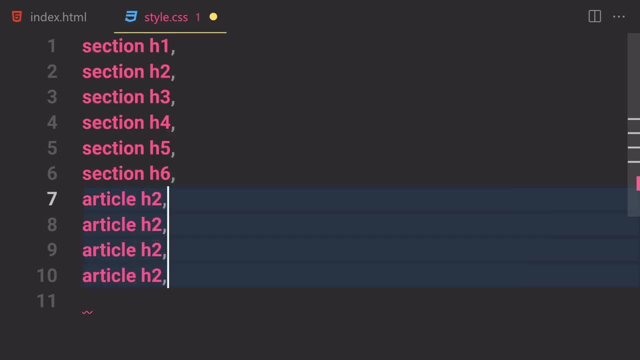 like article, and then h1, h2 and so on and so forth. so let's just write h2, h3, and then we are going to be using h4. and now let's just duplicate that two times, and then we are going to be using h4. and now. 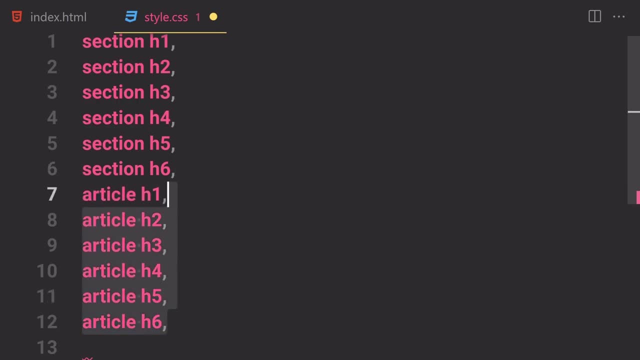 one more time. then we have h5, then we have it six. and now let's just copy that and paste it one more time. then we are going to be doing a multiple selection for uh, what do we call it aside. and now let's- i guess that would be fine- now let's just do multiple selection for uh, what do we call? 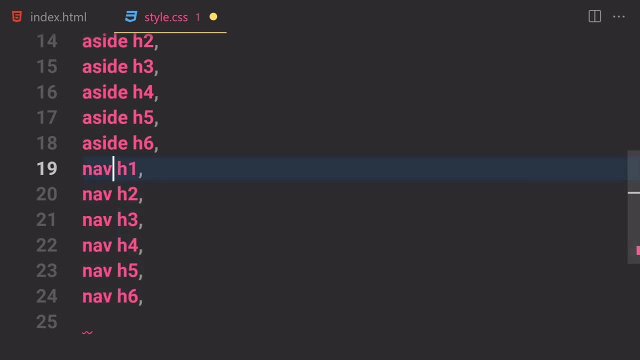 it navigation. so now we did a lot of multiple selection and stuff like that. so now, finally, we are going to be just using our curly brace right, and now i want you to just notice these selections. so we are going to be using h1- h6, then we have a article from h1 to h6, then we have our navigation. 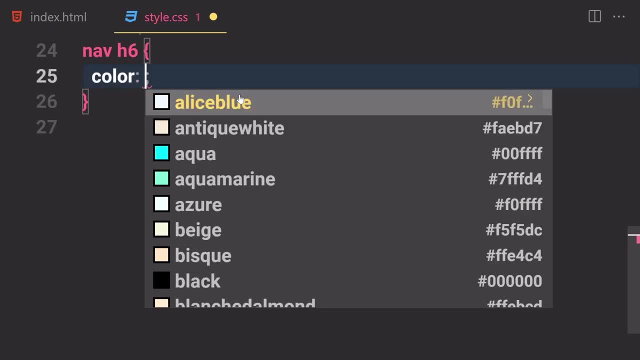 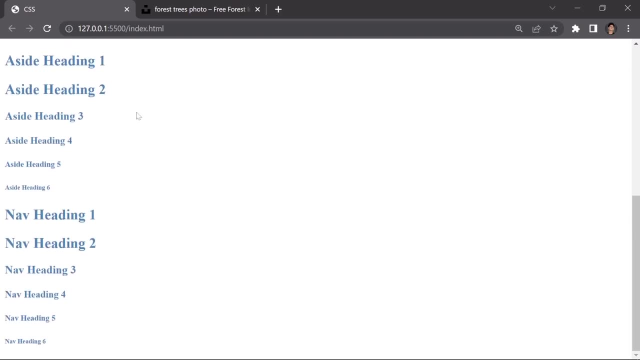 from h1 to h6, kind of crazy selector like that. so then, if you want to change the color to maybe like steel blue, and if you save that, so don't know- just provide that color to all of these uh headings right here. okay, just imagine the scenario like that and you will never have a scenario like this. 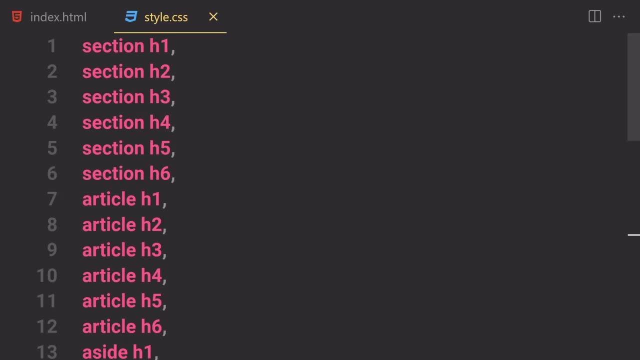 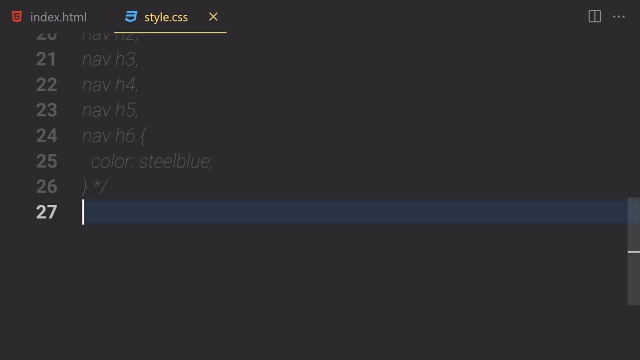 in a real world project, but i just kind of want to give you a example. so i want you to just notice all of that instead of writing. all of that we can use, or uh is selector, so i'm going to just comment all of the things right now and if you save that, we. 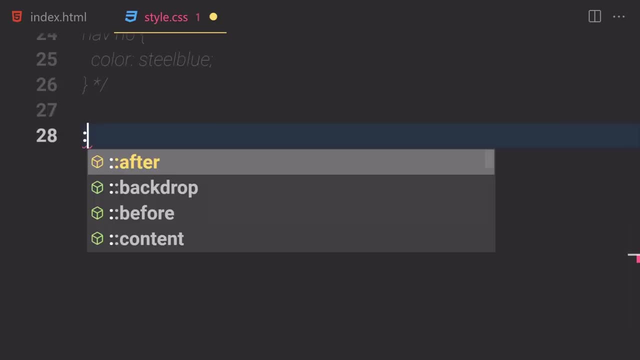 would get a, by default, a black color. so if you just uh, use a pseudo plus or a selector, however you want to call it, so we can just provide a section, then we can provide article, then we can provide a side, then we have to just provide a navigation and then now let's just use another is 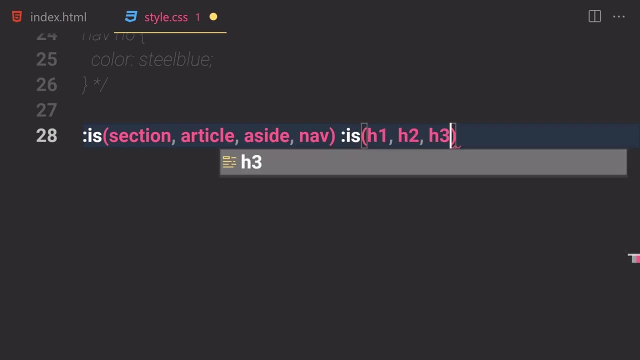 and here we are going to be using h1, h2, h3 comma, h4 and h5 and finally let's just use it six. and now inside there we are going to be using that kind of a steel blue color and knife is out there and boom, here you can. 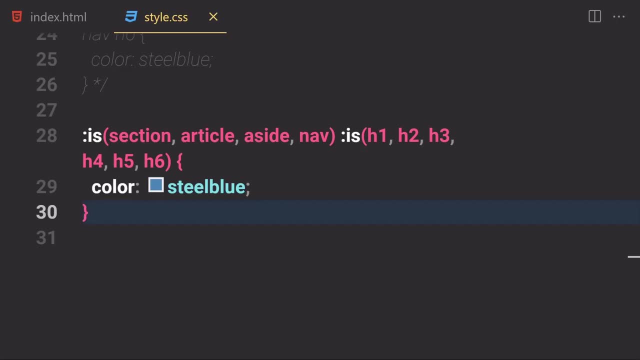 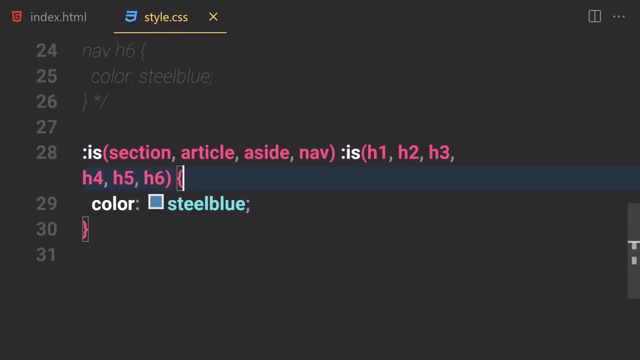 see it will now apply that color to all of its element right here. okay. so instead of writing all of these selector so now we can refactor our code to the selector right here. so if you zoom out of it then you can see the difference between like both of that right here. okay, so that was it about. 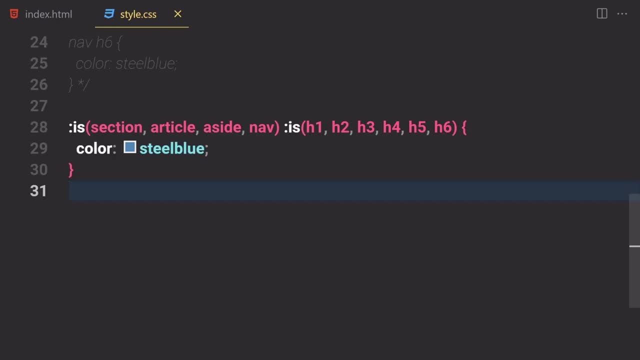 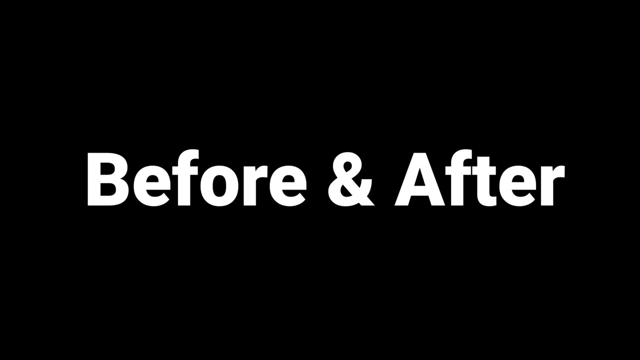 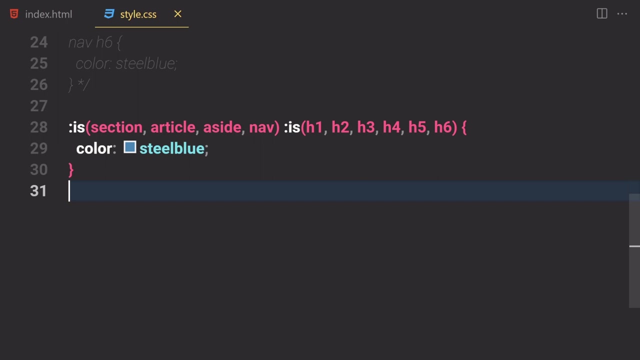 is selector. and now let's jump into a new topic which is called, i guess, a not selector. let's see which ones are predominantly used and which one is the most popular one. so now that we are totally done with the is selectors, now let's just learn about the. 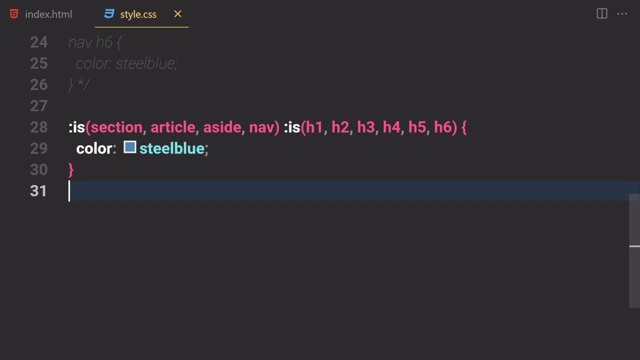 before and after a pseudo selector. but before getting into the before and after a selector, first of all let me just say this: these are crazy selector which can be used in a lot of different. it can be like before and after selector, totally guide. but i can't promise you that for now. but i 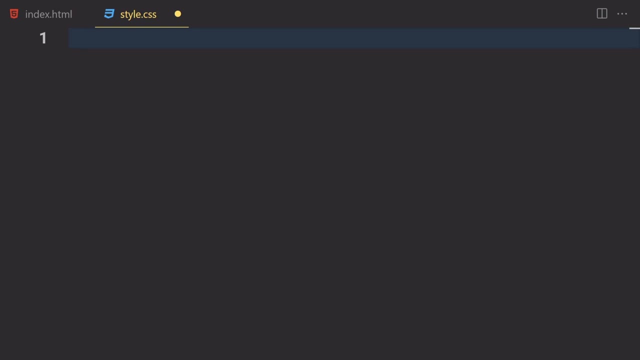 just kind of want to give you the test of that. so i'm going to just remove everything which i have inside my style sheet and i'm going to also remove everything inside my body right here. so totally clean body and totally clean style sheet. so inside a body i'm going to just write: 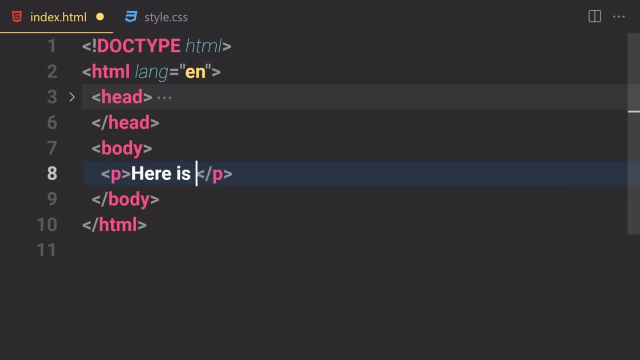 a paragraph and let me just write like: maybe here is uh some content right here, so i'm going to sell that and here you can see you're now getting like: here is some content, now let's jump into our css and now let's just tile there. so first of all, let me just center everything. first of all, i'm going 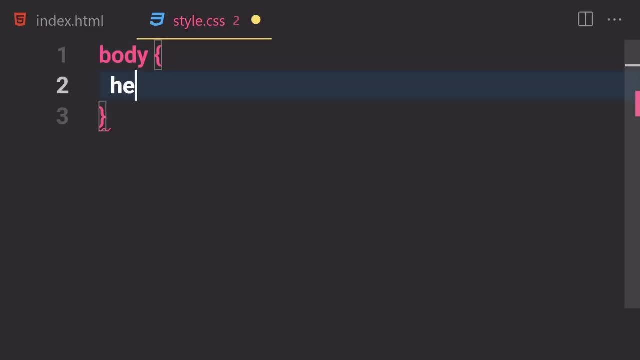 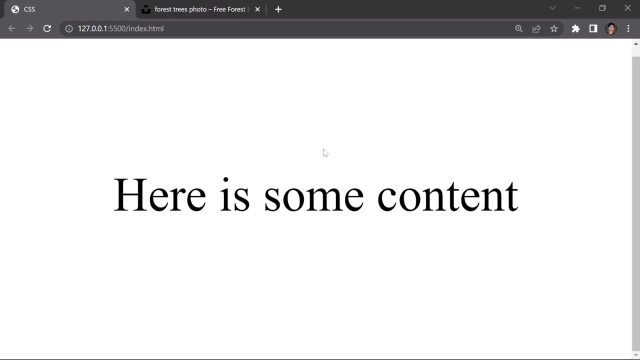 to write like a body. of height will be 100 vh. display will be totally flex. uh, justify. content will be center aligned items will be totally center and font size i'm going to put like fireframe for now and if you sell that and here you can see, everything is now totally at the center. 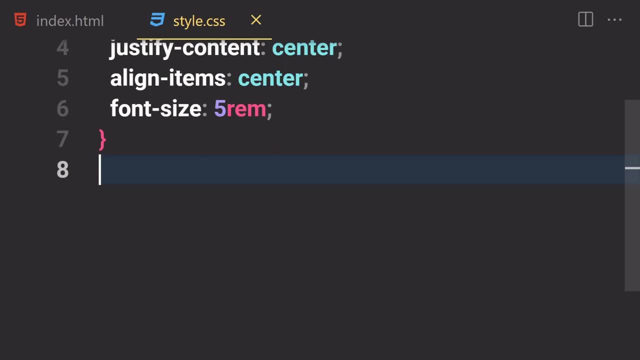 and or content is now taking like five frame of height anyways. so now let's just talk about something called before selector. so before selector insert content before a selected element. so, uh, the difference between the before selector and the after selector is that before selector insert item before the. 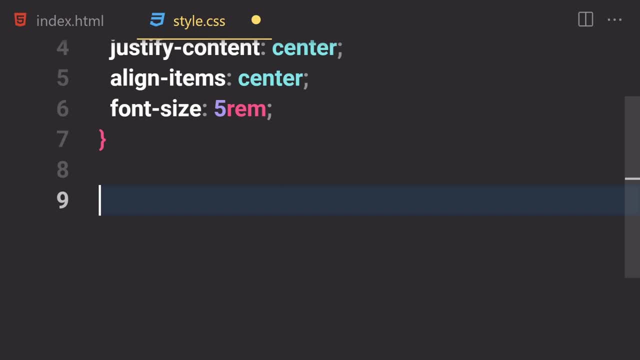 element after insert content after the specified element. so this selector can be commonly used, like to add some tags or anything you want. so i know that was just a horrible definition you i'll give you. so now let me just write some code and then you'll get to know what i'm talking about. 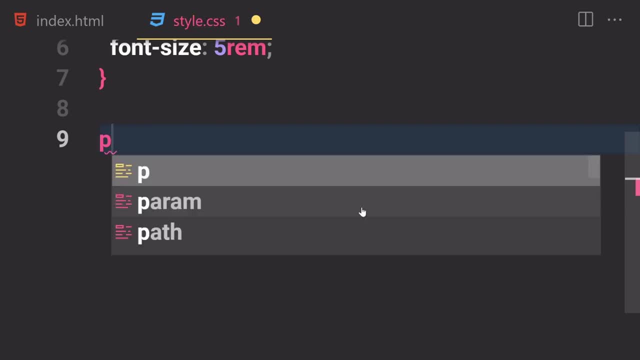 so if you want to use that, first of all you're going to be writing a selector name, then we are going to be using double colon right here, and then we are going to be using a before or after. okay, so we are going to be just writing before in this case, and now let's just. and now the next. 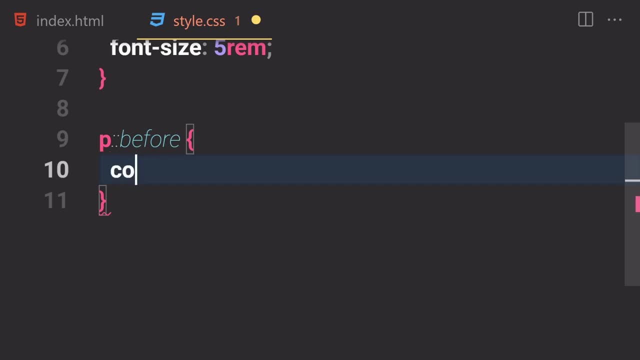 thing which you have to do inside this before we are going to be placing a content. okay, so if you want to put any content whatsoever, so you cannot like. if you want to put anything, so you don't have to put anything. so if do want to put something like maybe hello, so you just write a hello in here, or you can just put an. 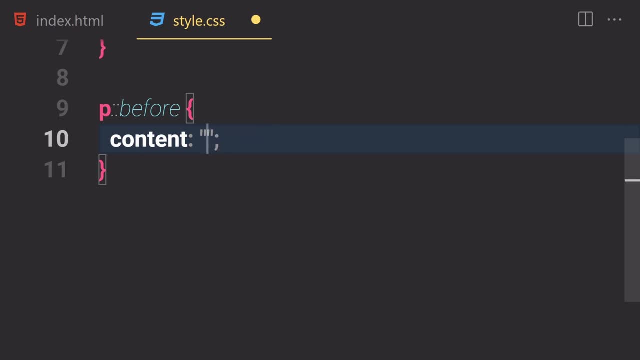 image. if you have image, you can also put like: maybe svgs, if you have svgs, you can put html entities if you have them. but in this simple example i'm going to just put like hello, and then we can just tile this content which we provide right there. okay, so we can just use like: 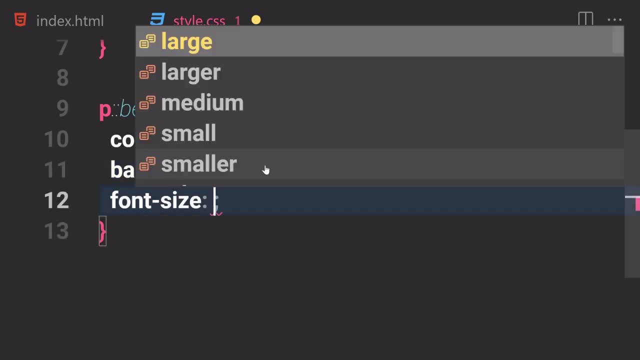 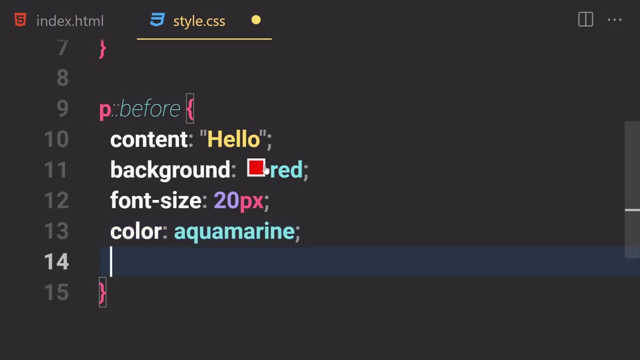 background color of maybe red, and we can also just increase the size of that, like maybe 20 pixel. we can also change the color to be like maybe, i don't know, let's just choose like this color and we can also change the font weight. if you want to so like, let's just write at 100 and if you sell, 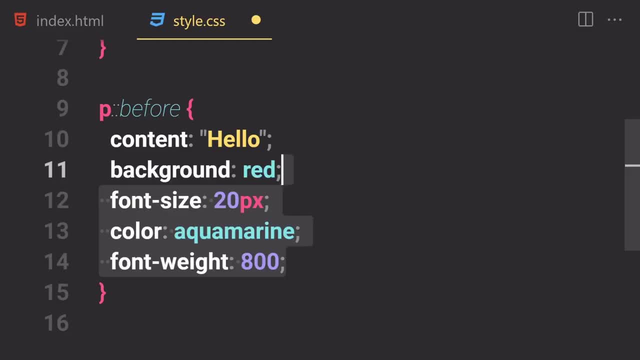 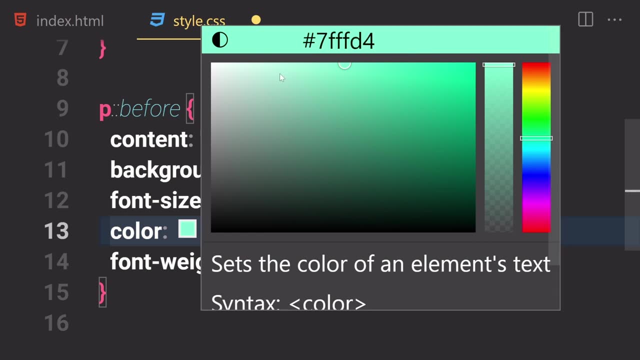 that, and here you can see it will now add this element right here. you don't have to provide all of these styles like you can choose whichever kind of style you like. you know, i'm going to change this color to be maybe like um, i don't know, i guess i'm going to just go with a totally pure. 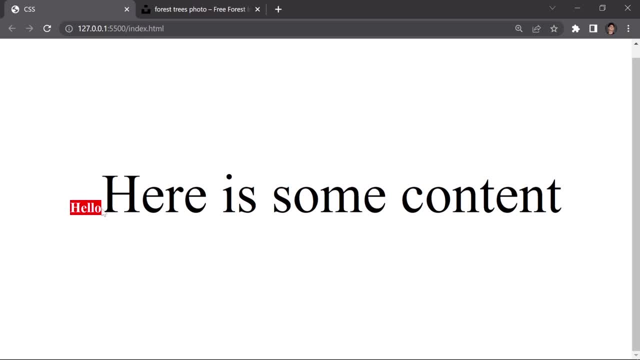 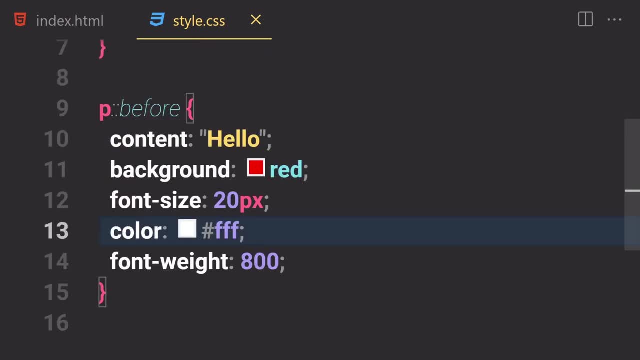 or white, and if you sell that, and here you can see we are now getting this. uh, hello, right here. okay, as i said that before and after selector can be used in a lot of different kind of scenarios, but this is just a quick example of before and after selector, so this is how we can put content. 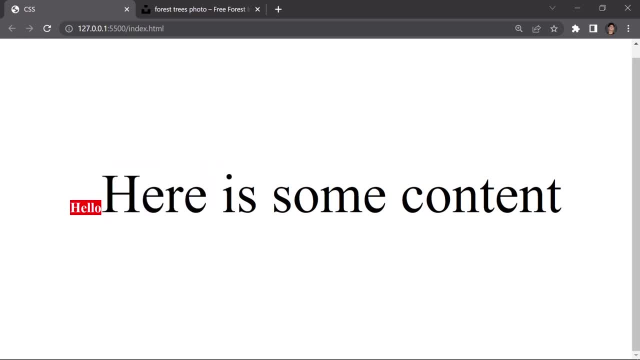 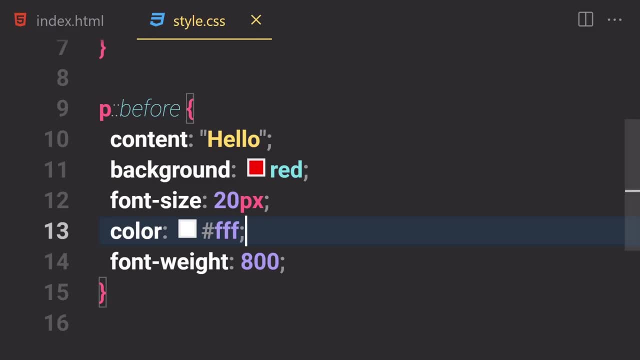 uh before the element. like we first of all have this paragraph right here and we want to put like hello, uh before this element. so this is how we can put that. if you want to put that content after that element, so for there, we can use after. okay, so now let's just select our p tag right here. 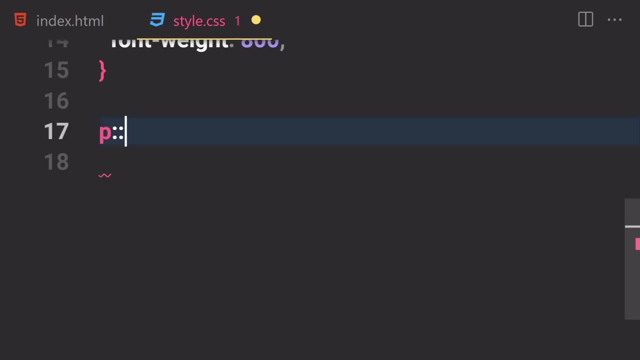 and now let's just use our double columns right there. and now let's just use the. so here we are going to be placing like content of buy maybe. and now let's just uh style that over. so i'm going to just change the styling to be red. the font size, uh, will be like 20 pixel. 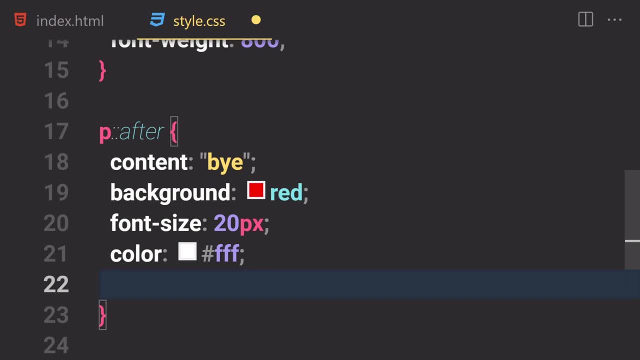 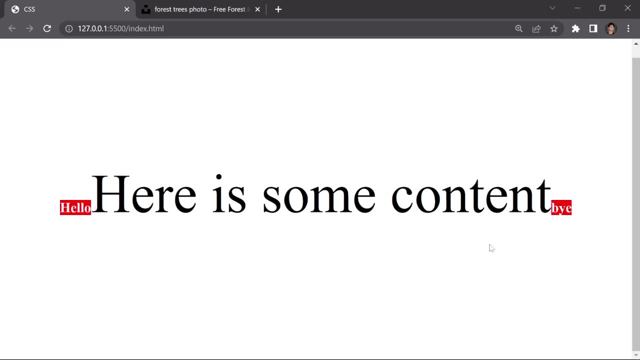 and the color should be totally white, not should be. i shouldn't have to say should be, but font weight will be just like: add 100 pixel, not pixel, but just add 100. so if you save that- and here you can see, this is how we can provide content before the element. 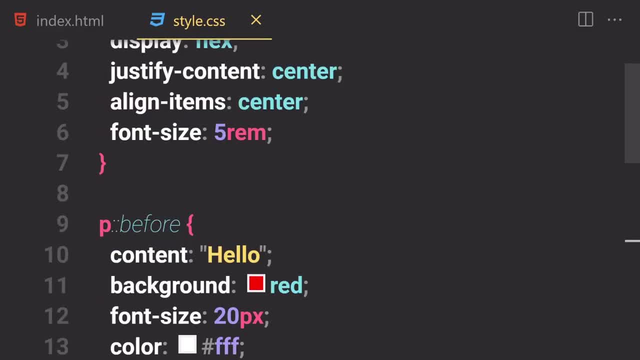 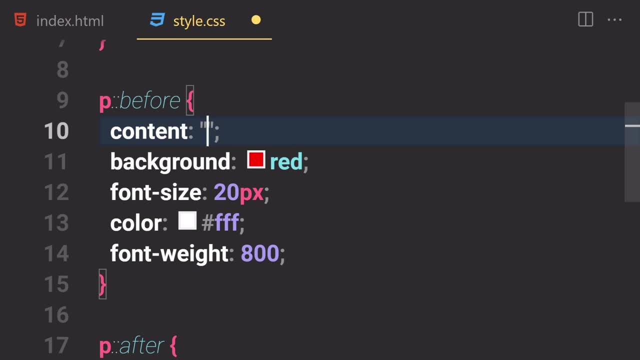 and this is how we can provide content after the element. so you can go crazy, like: instead of putting like hello, you can also provide like, maybe some. you can also put images, you can also put a font. awesome, as we learned in the previous videos. but in my case, i'm going to. 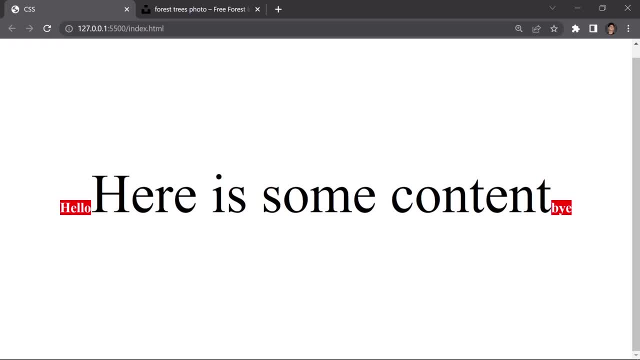 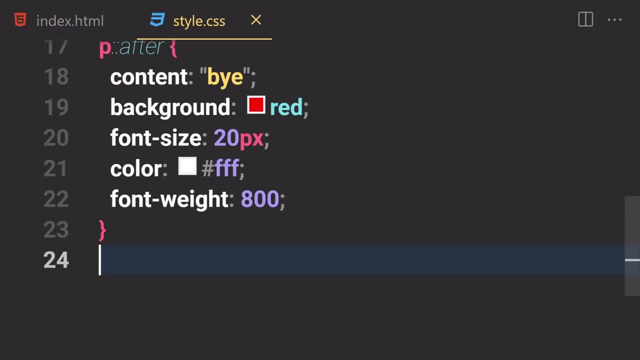 just put like hello and if you save that, so it will not give us hello and bye. so this is how we can work with that: before and after pseudo selectors. so now that we are totally done with the before and after selectors, so now let's just learn about a final- uh, pseudo selector in this go. 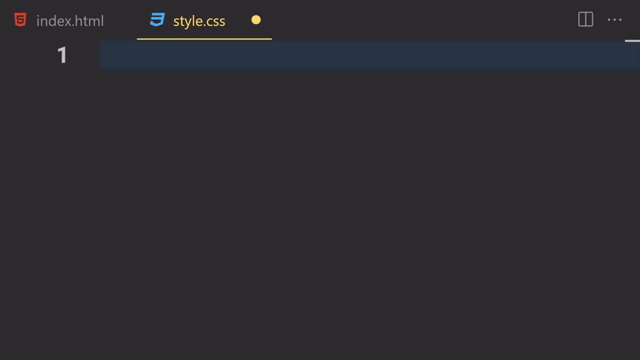 so now let's just learn about a not pseudo selector. so i'm going to select everything and i'm going to remove that in style sheet, and i'm going to select everything and remove that inside a body tag as well. so now, in this case for the not selector, first of all we have to write some 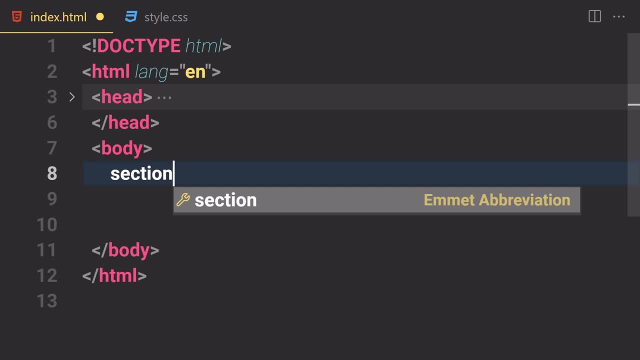 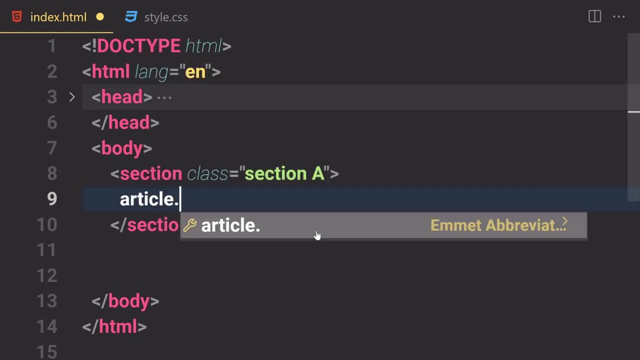 sort of html. so i can give you a cool example. so i'm going to just write a section with the class of section as well, and i'm going to also put an air right here, and then i'm going to provide like article with the clauses of article title. so i'm going to just put like article title. 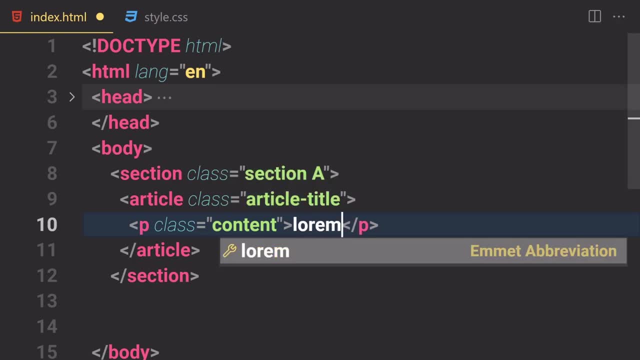 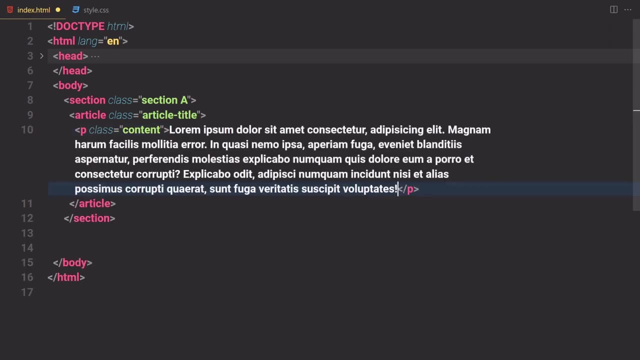 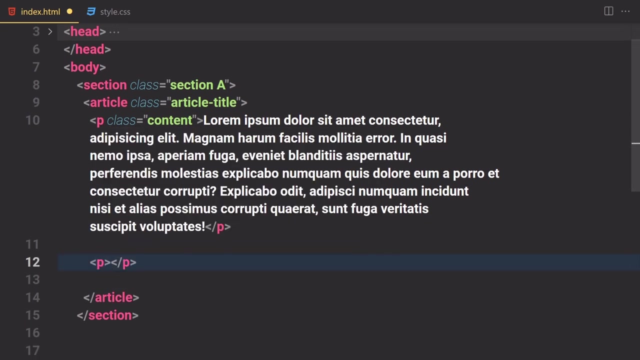 now let's just use a paragraph of content and i'm going to just put like lorem of maybe 100 would be fine. you know, lorem 100 is just uh, overkill. so i'm going to just go with like 50 lorem ipsum and that would be fine. and now let's just write a new paragraph right here and now let's just 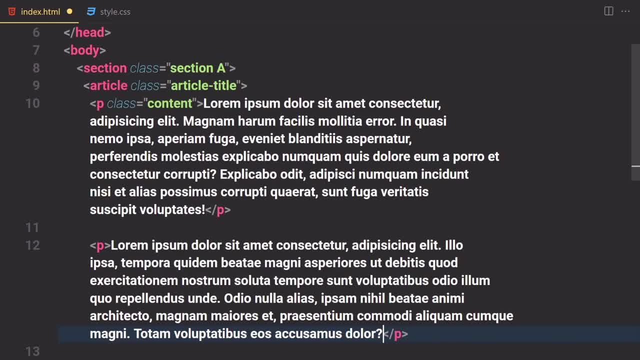 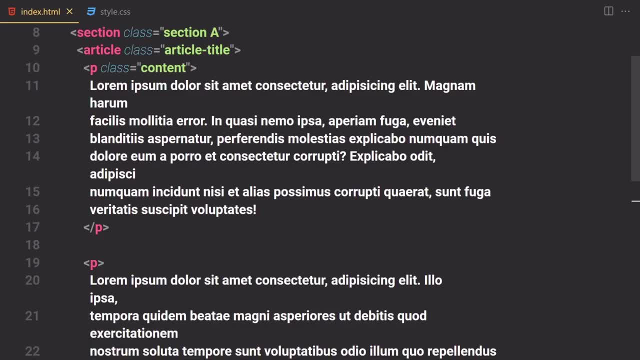 provide a lorem ipsum of 50 one more time. so i'm going to just put like lorem 50 in here and if you save that and we are now getting our lorem ipsum with the class of content, and like this lorem ipsum or this first paragraph will have the class of content and the second one do not have any. 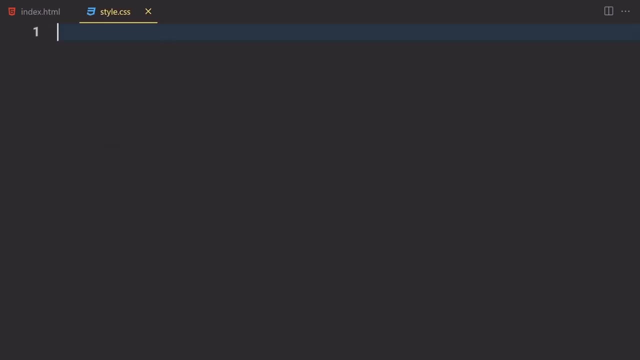 clauses and any ids and stuff like that. so now let's just get into our css and now let's just work on a not clause, so not not close, but not pseudo selector. the not selector matches every element that is not specified in that element selector. so you know what? first of all, let me 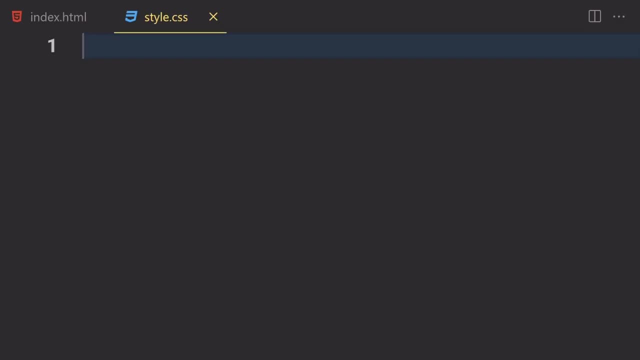 just write some coding, then you will get to know what i'm talking about. so first of all, let me just get my section and i'm going to put a width of like maybe four or five hundred, and i'm going to put a width of like maybe 42 rems or not rems but m, and i'm going to also provide a margin of zero. 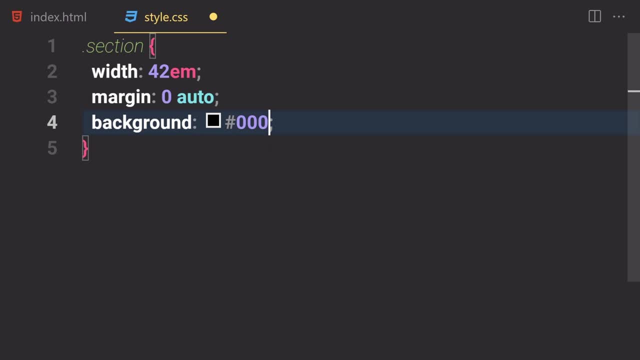 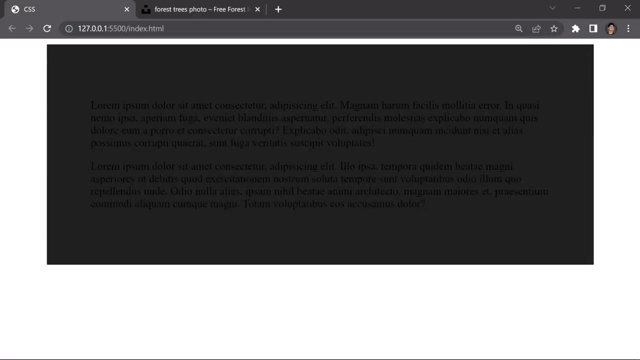 auto, so that our content is now at the center. let's just provide a background color, to be like maybe rgb of uh 32, 32 and 31. okay, so now let's just put a padding of four rems in this case, and if you save that, and this is how currently our content looks like and you know what i'm going. 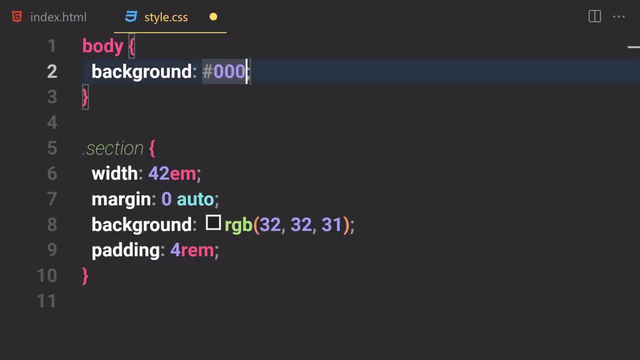 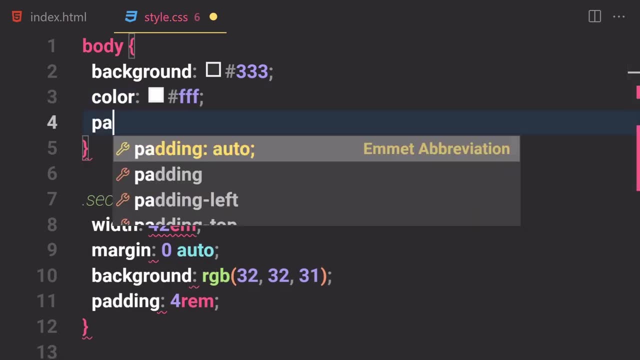 to just select my body in here and i'm going to put like a background color of maybe 333 in this case, and the totally. the color will be totally white and i want to also put a padding of two rems. so if you just sell that and this is how currently or content looks like right now, okay, so, 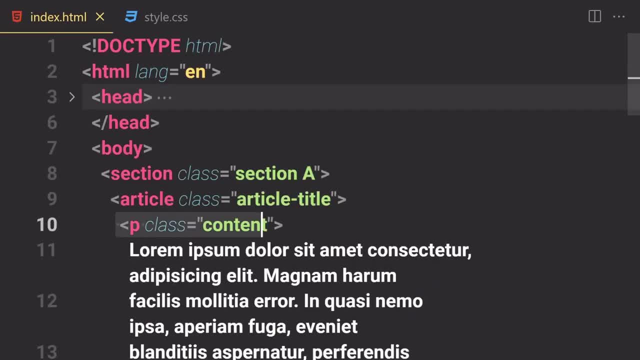 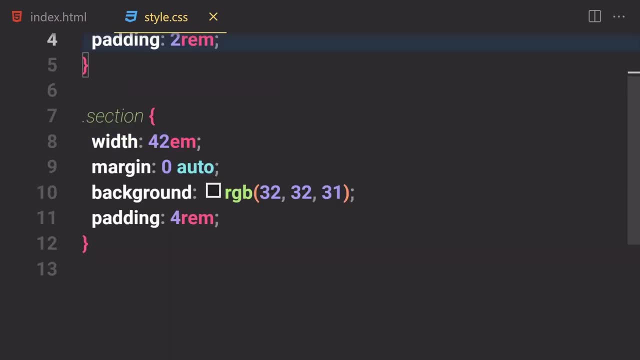 now here, i want you to notice that in this class, in this first paragraph, we provide a clause of content, but in this second paragraph we didn't provide any clauses, any attribute, any stuff like that. so i want you to just notice that. so now, in this case, we want to select like: first of all, let 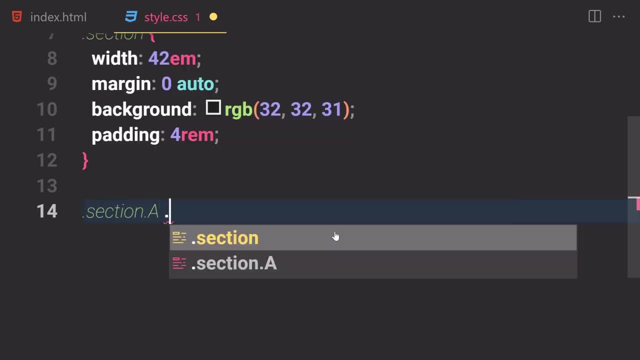 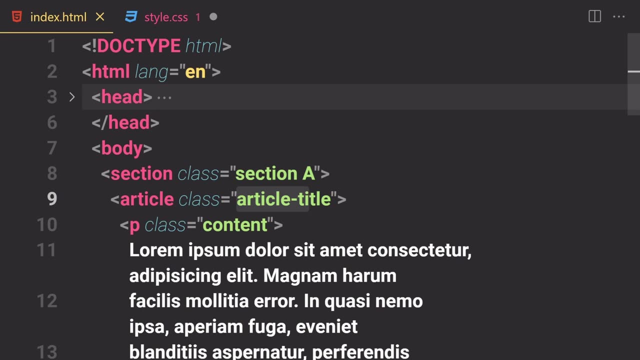 me just write a section and now let's go ahead and put that. so let's just put this class here and now just get our a, and then we have to get our article uh- title. so we are now inside this article title right here. so you want to do a little bit of nesting in there. so we are now just select word. 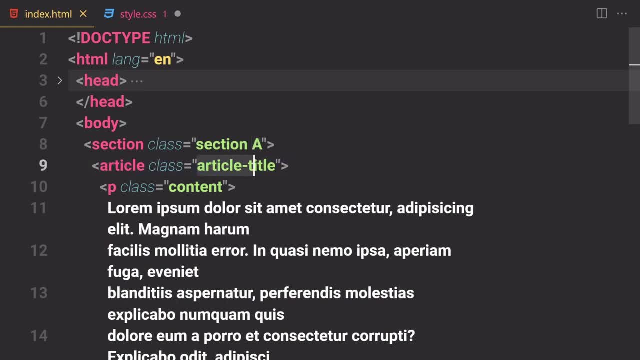 section, then we select this spirit section, then we select word section or not section, but just article title or you know what. we can just remove this a from there. we don't need that. i just kind of want to give the example, but we don't need that. so simply just remove that. so we would just 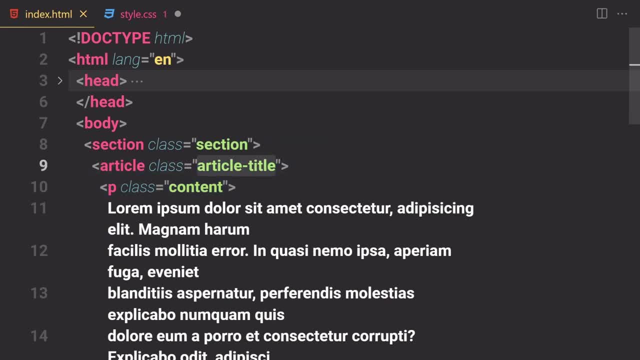 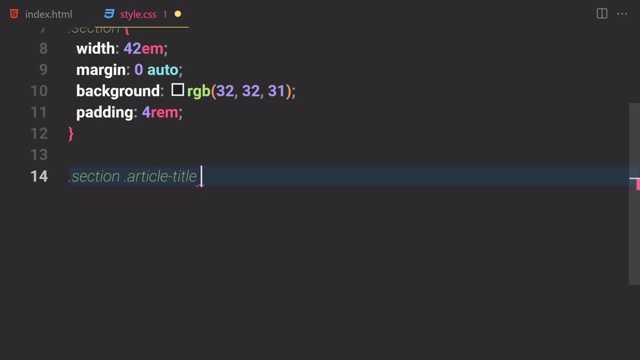 select word section, and then we are going to be just selecting this section or not section, but article title. and now let's just, you know i'm going to provide a space in there and now let's just use that, not a pseudo selector. so if you just write not, and then we just provide a content in 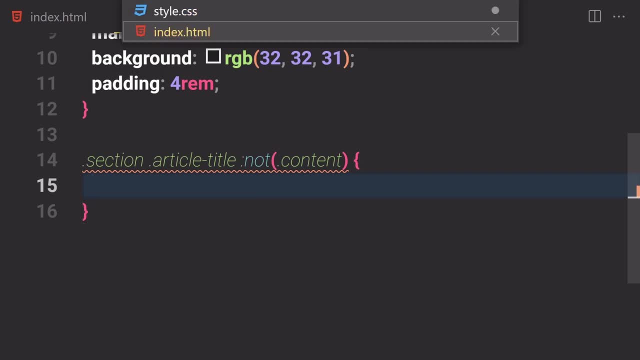 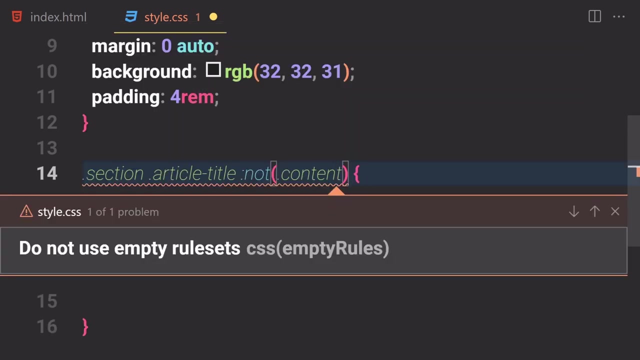 here. so now let me just provide a content. so we are now selecting this content class right here. so any style we apply to this selector, like we select word, section, then article, and we specify not, so it will just skip that and it will provide that style into all of their elements. okay, so all of their selector, all of that selector, will be specified. 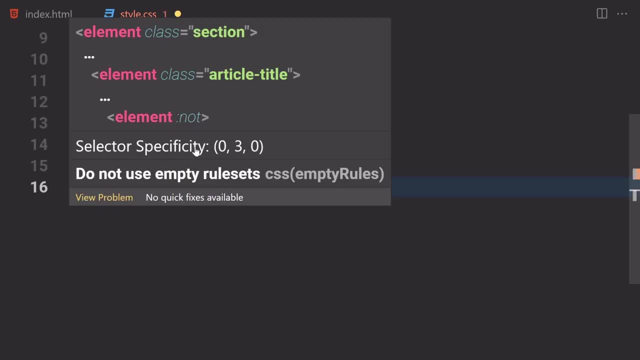 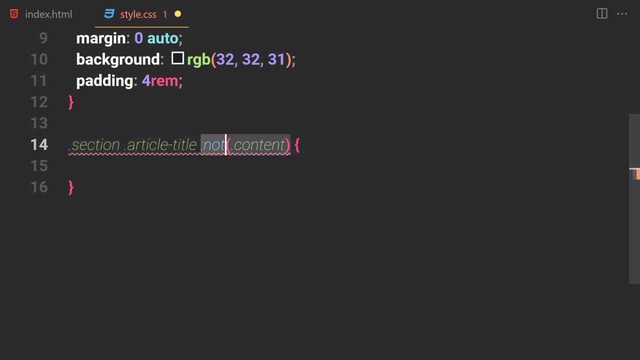 oh, my goodness, what the hell am i doing? so go back and it will now. it will now specify their styling to all of their selector, which we select already, but it will just ignore or it will just skip this one which we provide inside this. not so to selector. now, let's suppose if you want to give. 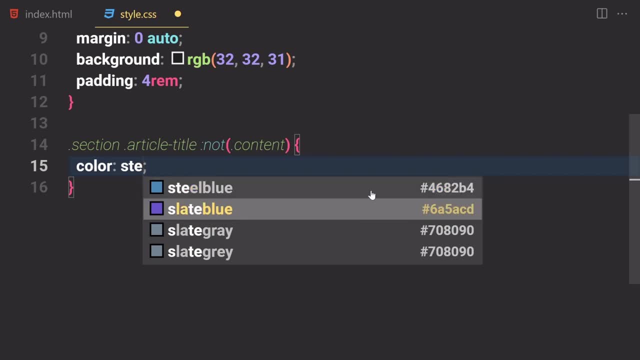 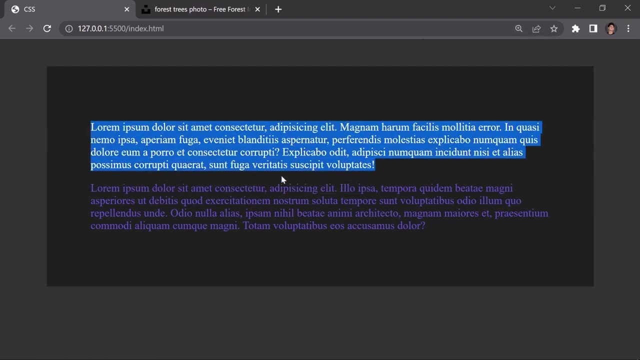 a color of like. maybe steel blue or slat blue would be fine. and now, if you save that, so here you can see, it will give you a color of like. maybe steel blue or slat blue will be fine, and it will not provide color to this content class, but it will do provide color to the second class. 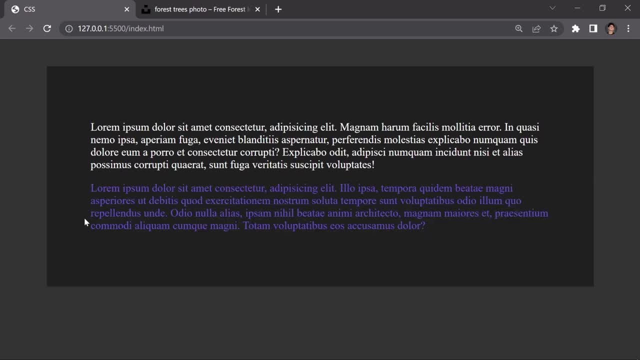 right here. so if you have like maybe thousand more paragraph tags, so it will just provide that colors to all of them, except which have the class of not uh, i mean like which have the class of content. so if you just right click on that and go to the inspect, so let's just write f12 in here and now. 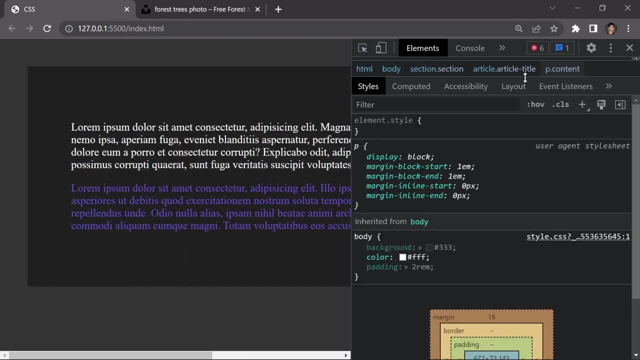 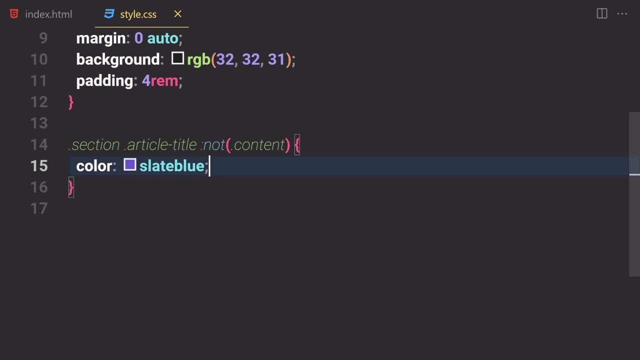 let's just select our first one. so let me just show you that real quick. so here you can see this. here is the font size, which is the font size you just can, hurting the font size. you know, cover up the layer type a minus the font size, right here, and we specified that in word. 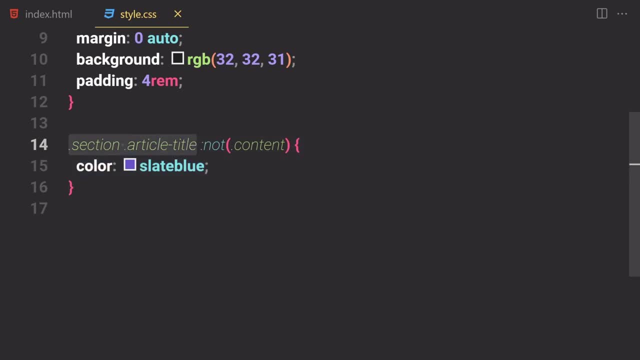 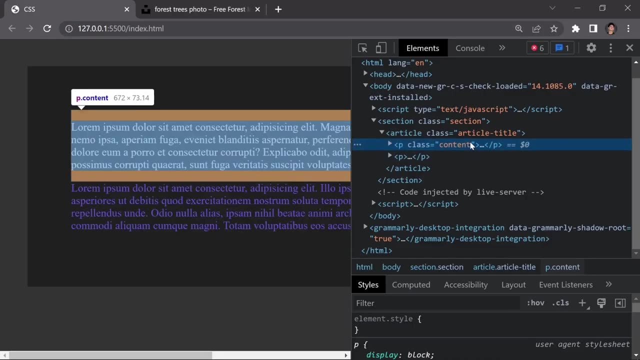 not selector right here. so we want, so you want, to provide this tiling which we are going to be writing inside this curly braces. we want to apply all of that style to all of that element which we first of all have, but just ignore this one which we selected inside this not class right here. okay, 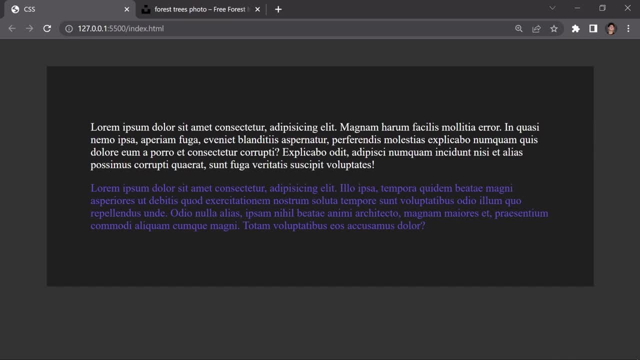 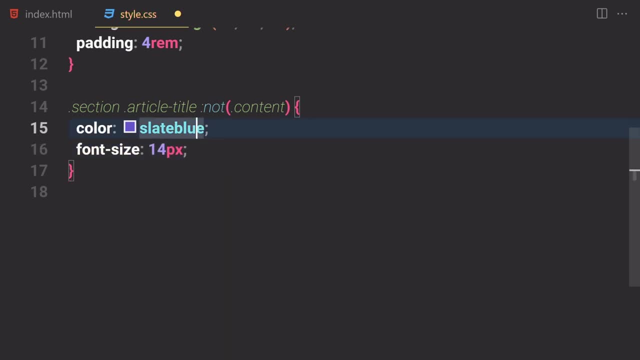 so this is kind of a cool anyway. so now let me just give you another example of that. so we can also just remove that nesting if you want to. so now let's suppose, if you want to increase the font size, тыس над use a font size of 14 pixels and now let's just remove these article class and these a lot of. 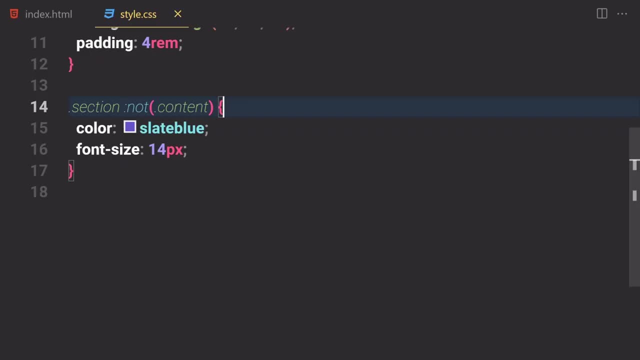 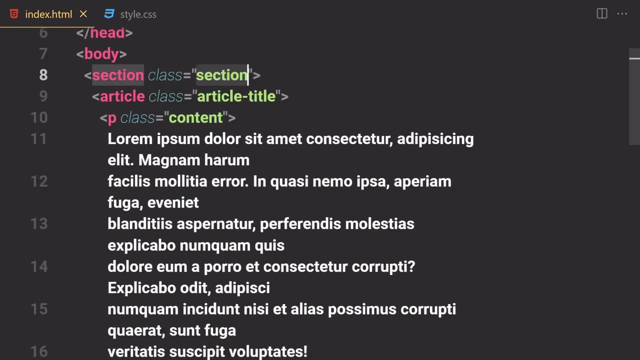 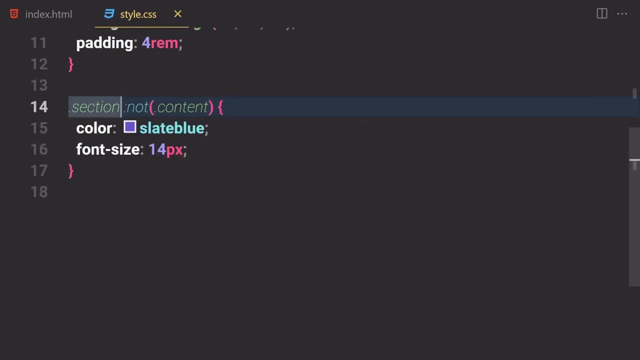 nesting, so you can just remove that and if you save that, and i guess we messed up something. so we are now selecting word section. uh, okay, so we are now selecting this section and then we are selecting all of their content. so that's not, that's not a great idea. we have to put that article one. 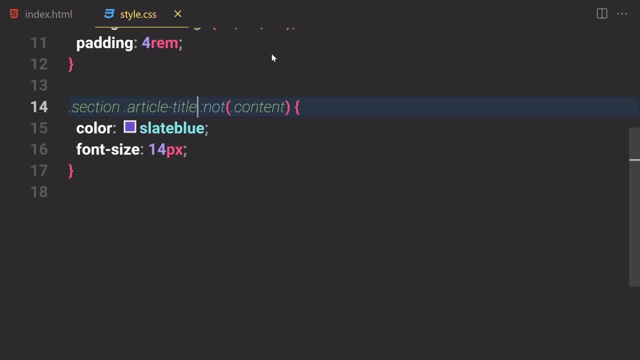 more time so you can just use article title in there. so if you save that- and now this is how it works. so this was just a first example of that- not operator or not. why am i saying not operator? this is the first example of a not pseudo selector. now let me just give you another example of that. 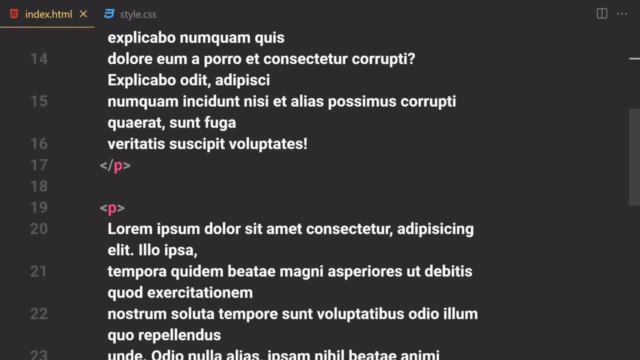 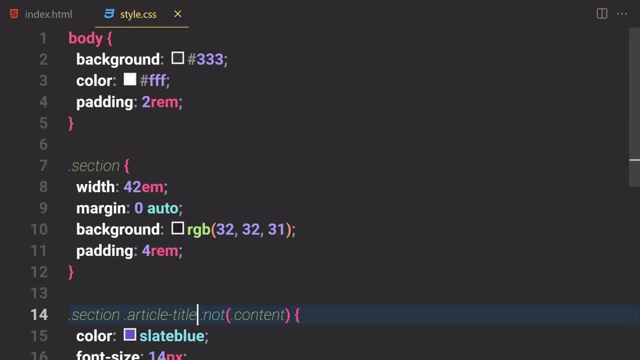 so for that we have to write a little bit more uh, html, or you know what? we have to first of all remove this example. so i'm going to remove this example from here and save that, and we also have to remove this example from there as well. well, you know what? we're not going to be removing that? 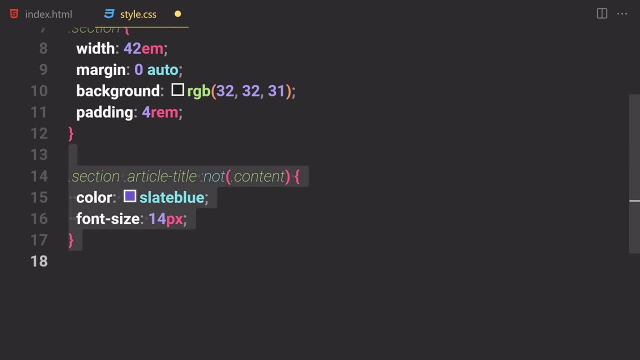 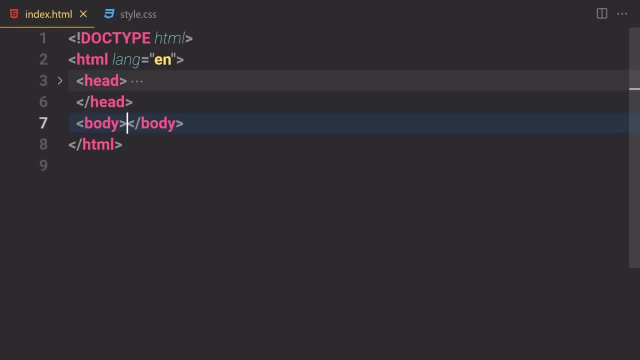 so we are going to be just removing this section and then article title and then that not operator. so i'm going to just remove that. and this is how everything looks like by default and you know what? i'm going to give you an example of buttons. so i'm 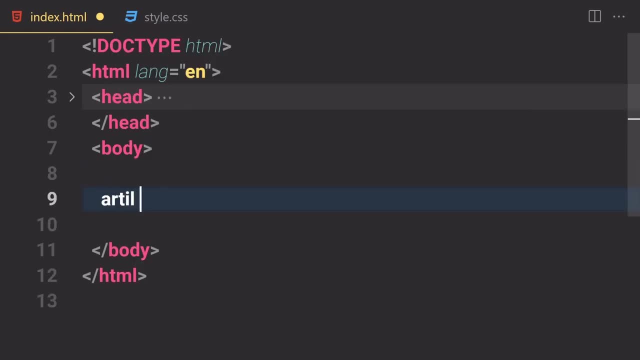 going to zoom in a bit and here i'm going to just create a new article: right here, our article, and inside this article. what do we have to do? i'm going to give them a class of like, maybe section in here, so you want to provide that section class which we already styled right here and inside this. 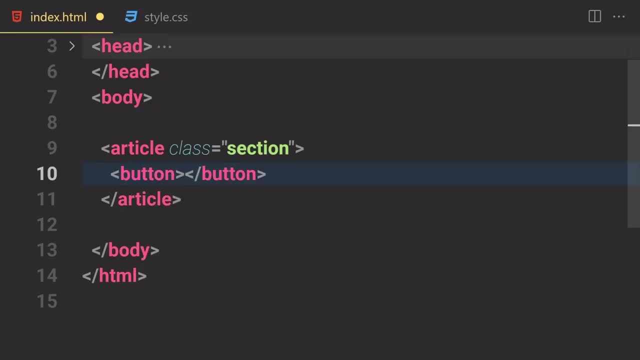 section. we have to just create a button, and now let me just write like button a, and now let's just duplicate that. we have button b, and now let's just duplicate that, and now we have button c. but in this case i'm going to provide a class of or not class. but 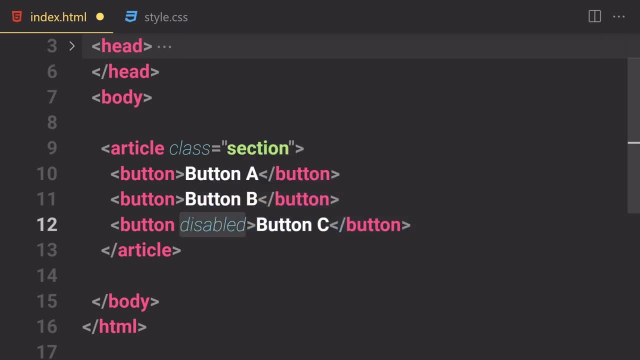 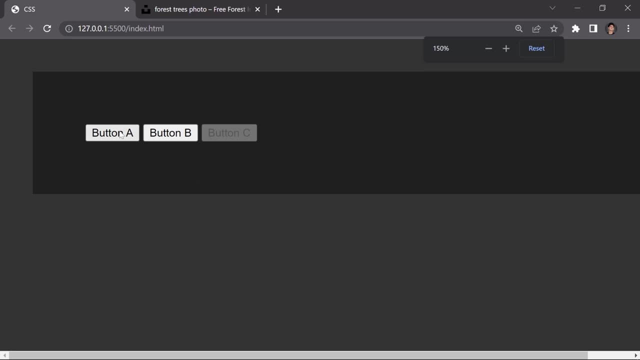 an attribute or disable. so if i just provide the attribute of disable, so if you save our file and this is how we get by default right now. so if you want to style all of these buttons, like this button a and button b, and if you want to skip the styling for this button c, um, which has the 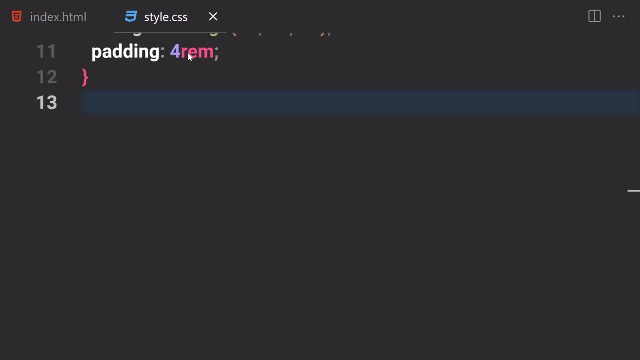 attribute of the. so if you want to skip there, so we can just write a code for that. if you want to, so we can just use first of all: um, so for that we have to use a section, and then now let's just select all of the buttons. uh, so i'm going to just put a button in there and now let's just use that, not a pseudo. 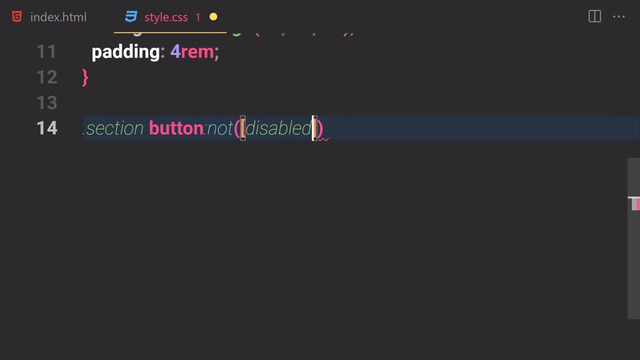 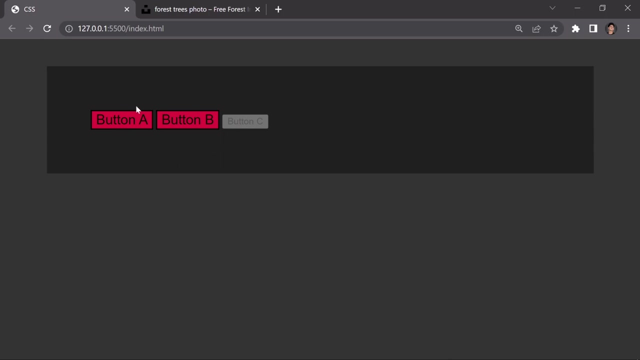 selector, and here we are going to be just specifying the disable d-a-s-a-b-l-e-d, and now let's just use like font size of 20 pixel, and now let's just use background color of crimson. so if you save that- so now here you can see- it will now apply all of that style to all of the buttons. 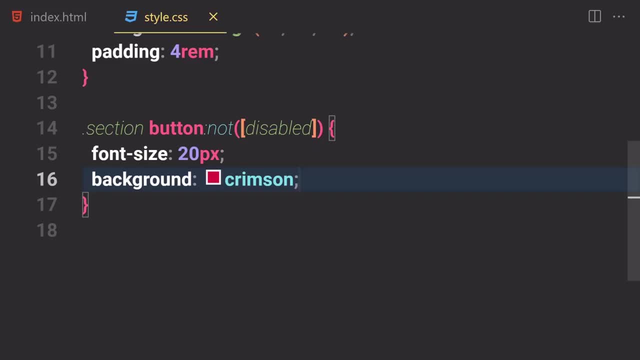 except this specific button, which have the class or not a class, but the attribute of disable. okay, so it will just ignore that. so now let me just give you the last example on the not pseudo selector. so i'm going to just remove that from here and i'm going to also remove this everything. 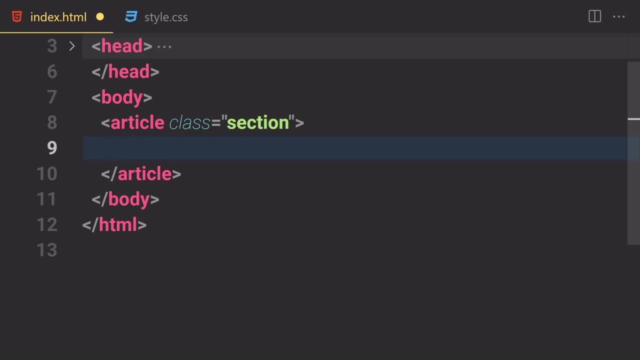 from this article as well. now let me just write like: maybe anchor tags. in this case, i'm going to just write anchor tag which will go to like: uh, i don't know my youtube channel, so https, and i'm going to just go to like: i don't know my youtube channel, so https, and i'm going to just 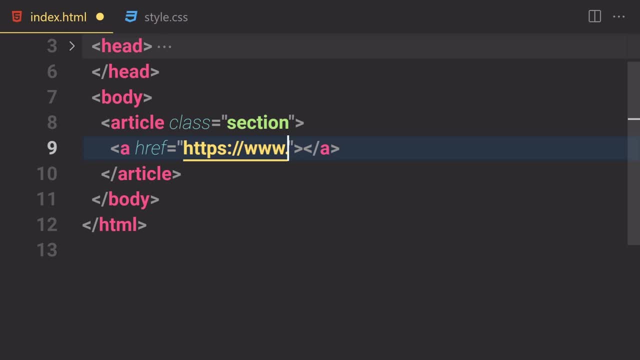 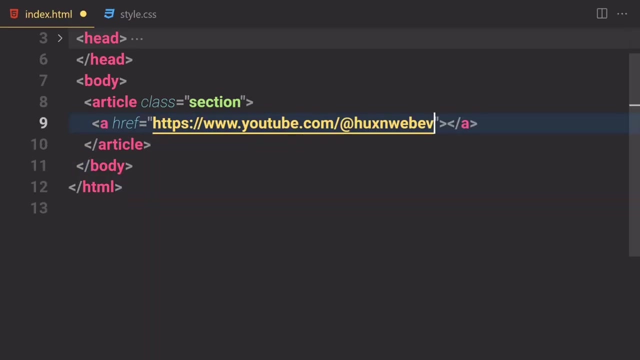 and then double slash is wwwyoutubecom. do i spell it correctly like u-t-u-b-e? okay, so y-o-u-t-u-b-e dot com. forward slash: zen web dev, my own channel. so i just kind of want to give you example of these anchor tags and i want to put like maybe yt for youtube. so now let's just select this second. 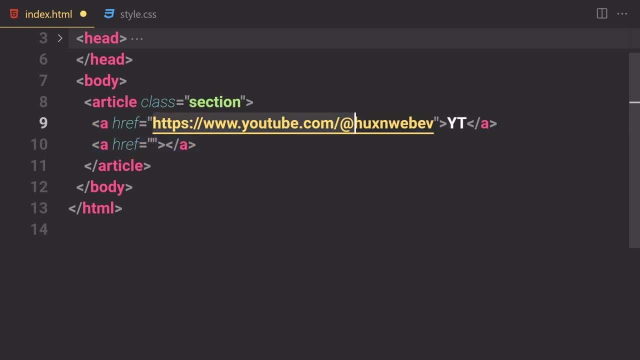 one. and what do we have to do? i'm going to copy this link from here and now let's space this link right there and i want to put like udemy right here and then let's just use like user of zen web dev. and then let me just put a udemy in here and duplicate this line of code, and here we have. 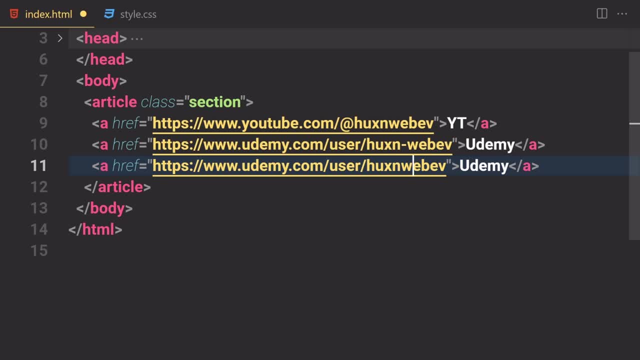 to specify their dash in there. and now let's just write like: maybe googlecom. so i'm going to just write like googlecom and i'm going to remove everything from there. so here we just have to replace that name you to google. so if we select that and save that, it will now gives us these three anchor tags, right. 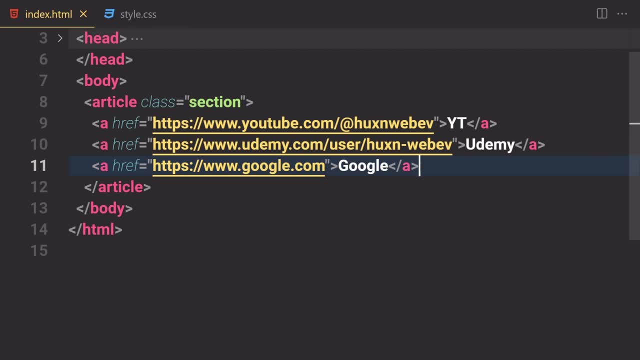 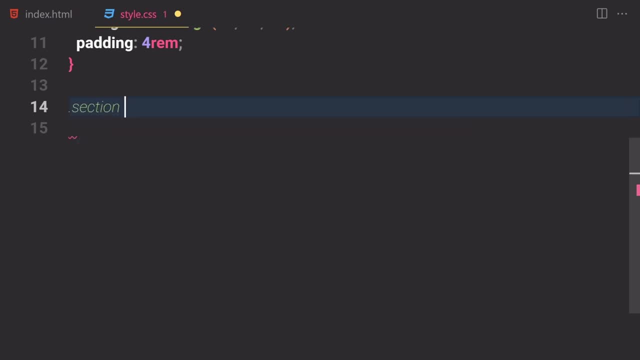 here. so if you want to style all of them and you want to just, uh like, skip one of them, so for that we just have for a little bit of coding. so now let's just select word section and now let's just select all of the anchor tags and now let's just use or not operator. but now, in this case we are. 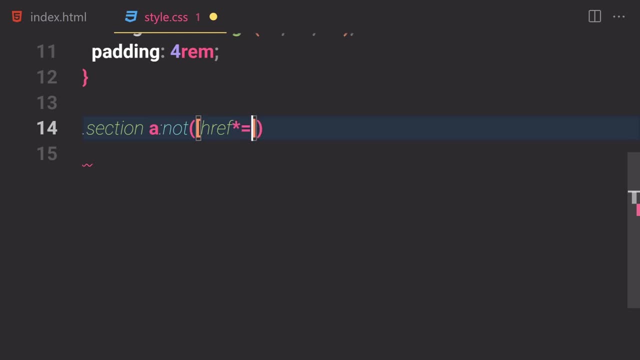 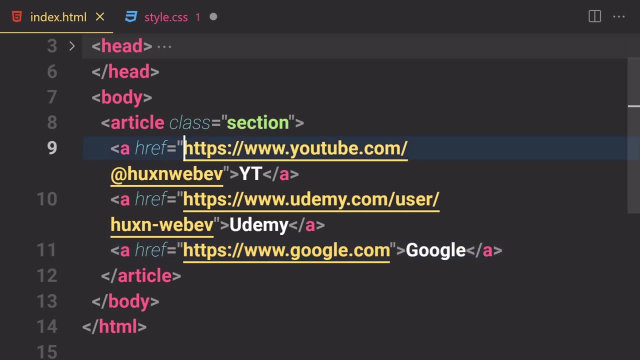 going to be using, or href, and now let's just provide this s symbol, and now let's just search for the one we don't want to style. so which one we don't want to style? it maybe like this youtube channel. so if you don't want to style that one, so i'm going to just paste. 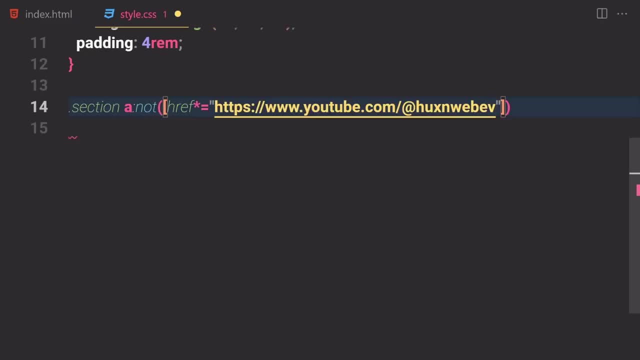 this link right there. so i'm going to zoom out a bit and this is how we can select that. and now let's just use our curly braces right there. and now, here i'm going to just provide a color of, like, maybe brown. uh, yeah, i guess i will just go with the brown color and text decoration i want to. 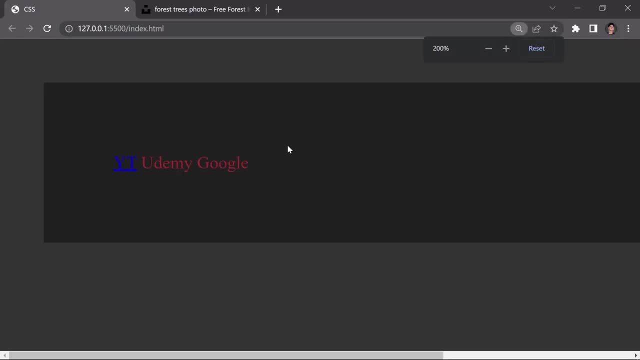 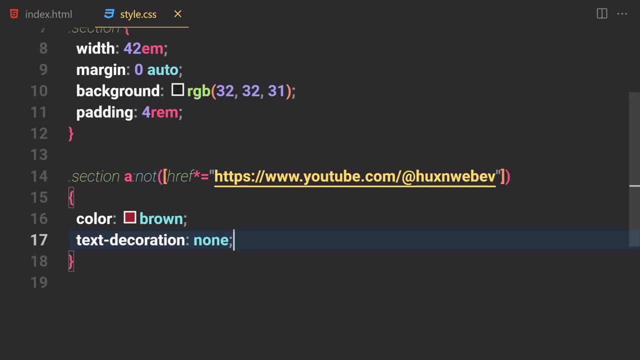 remove and i'm going to set that to none and save our file. so here you can see. it will apply all of their styling to all of these anchor tags, except this yt or youtube. that's because i'm going to just copy that and i'm going to paste this link right here and if you save that, so here you can. 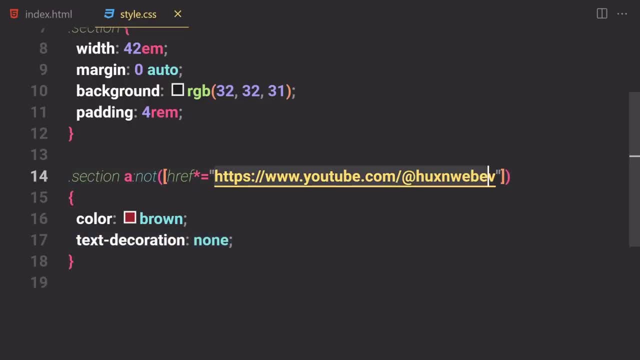 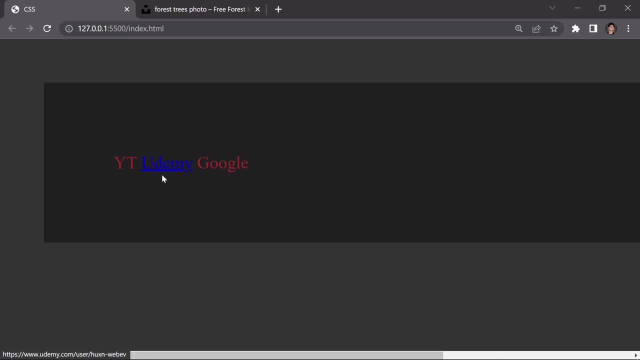 see it will not apply their styling to all of their anchor tags except this middle one. why that's because we selected that right here. so this is how we can use a node pseudo selector in css. so i'm going to just remove everything which we have inside word style sheet and i'm going to also 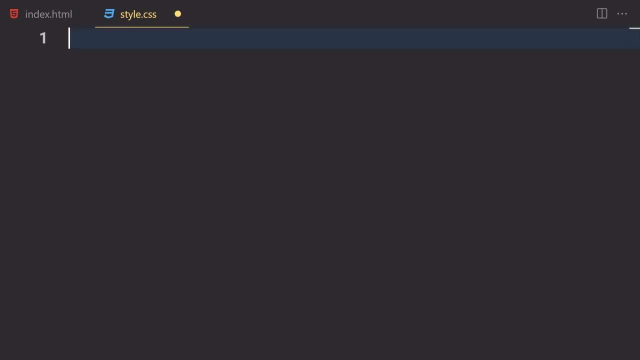 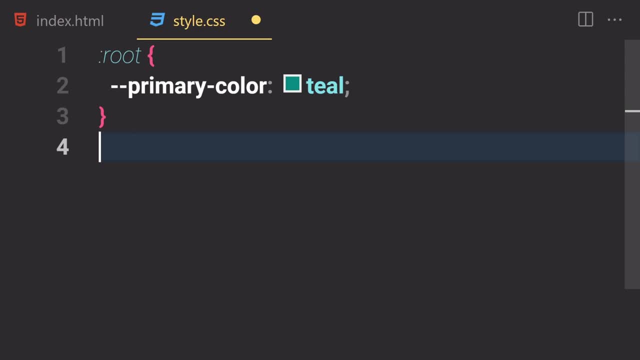 to also remove everything inside our body. okay, so we get our totally standard style sheet and i'm going to also remove everything inside our body. okay, so we get our totally standard style sheet and i'm going you use this variable. so now let me just give you example of like h1, and in here i'm going to just 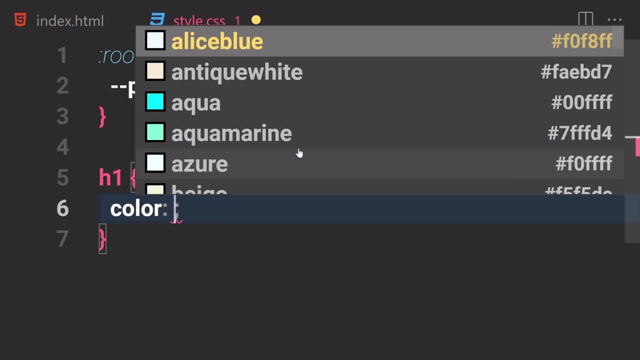 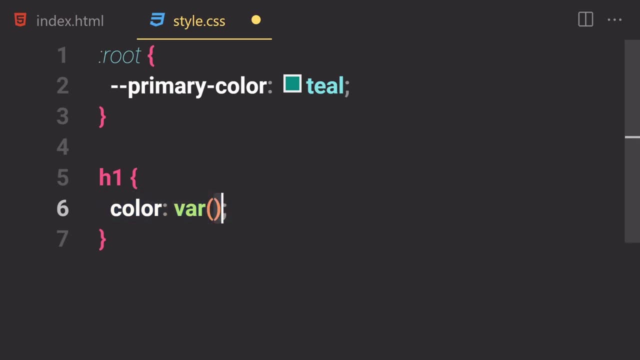 put like color. and now, if you want to use that variable, so what do you have to do? first of all, you just have to write a var, and then a var is a function. so for there, you just have to write opening parenthesis and then the closing parenthesis and then just name of that variable. 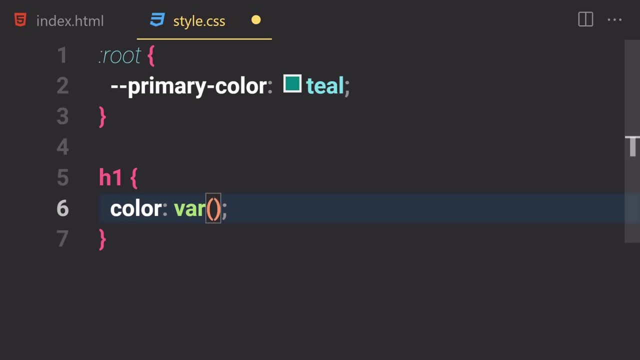 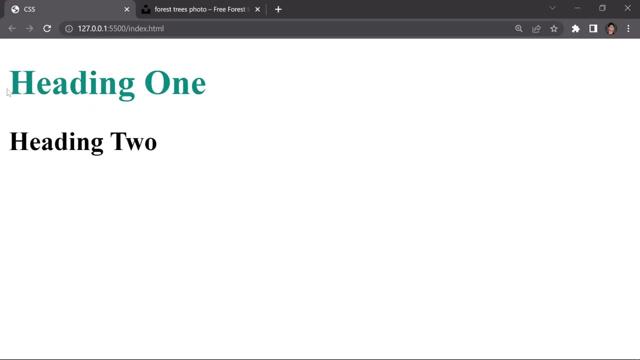 so which kind of name is or variable? or variable is now double dashes, primary color. so if you just select that and if you save that and here you can see, it will now change the color to teal color. so if you want to change this color, so we just have to go to our variable section right here and we 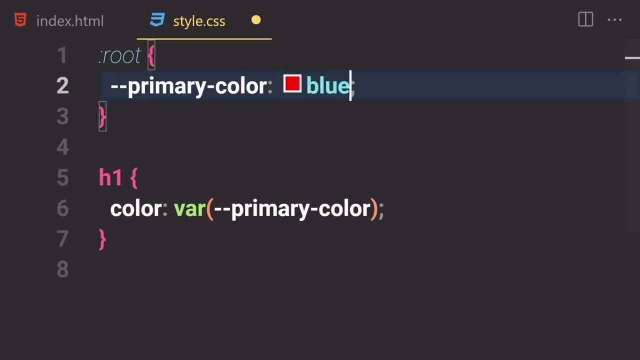 can change it to like red or blue or green or whatever kind of color you like. so save it there. so it will now just change it to that color. so i'm going to just stick to their teal color. now let me create a new variable. so let's just write like dash, dash of size, or you know what. 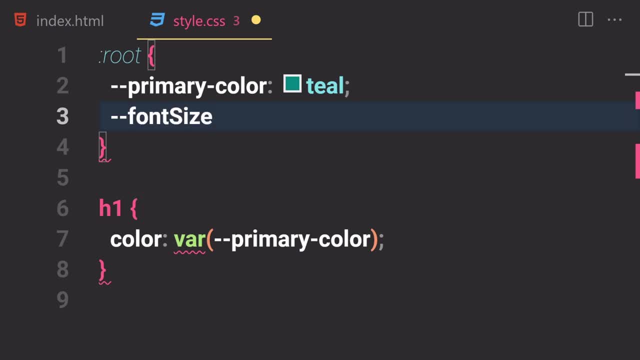 i'm going to put like maybe font size, or we can write it like camel case, if you want to, or we can just separate by a dash. so now let me just write a font size, and here we have to just specify like four rems right here. so now, in this case we want to select our h2, and now let's just increase the. 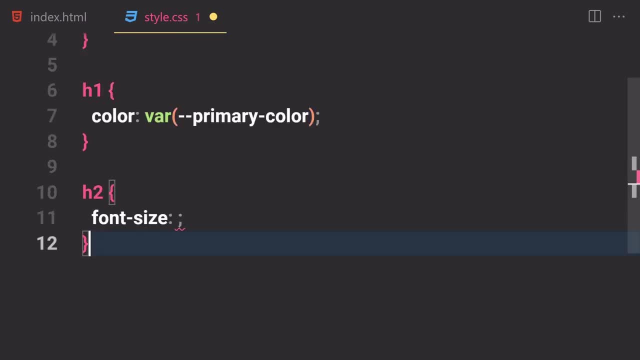 font size of their h2. i'm going to zoom out of it, and now let's just use our css variable. so now, in this case, we want to use the second- or not the second, but the first- variable name. so we are going to be just using font size. and now, if you save that and boom, here you can see the font is. 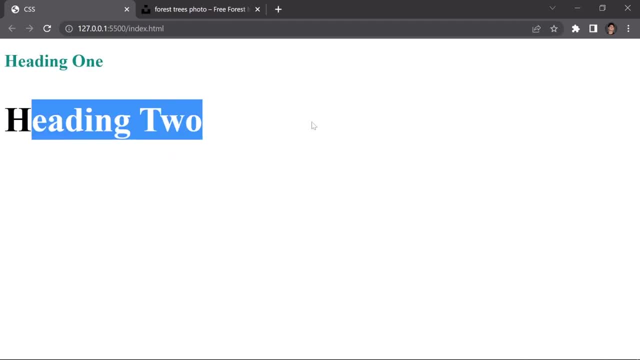 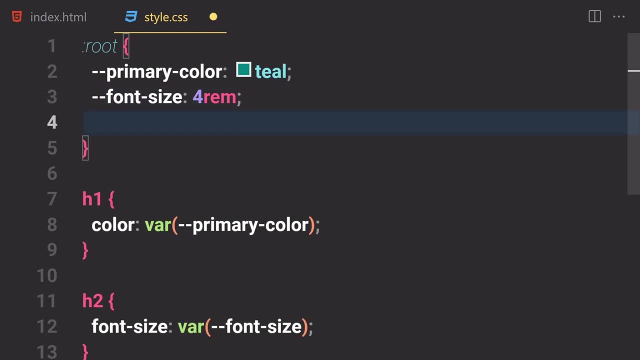 increased to like four rems, and now here you can see that, so we can create like countless variables for our project. but we will just keep things simple. so we just learn about colors, the fonts, and now let's just provide like, maybe bg color for a background color, and now, if you just use like red and red, 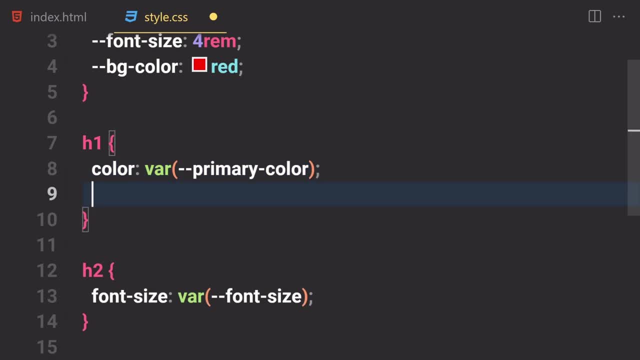 will be the kind of the background color. so now if you want to use the background color of this h1 to be like red, so we can just use like bg and we have to specify that war and then just use that sort of a color. so we. 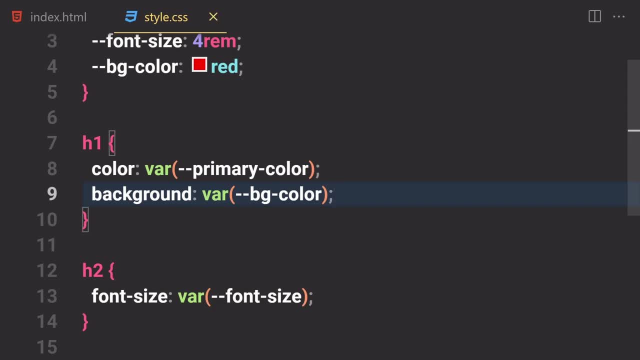 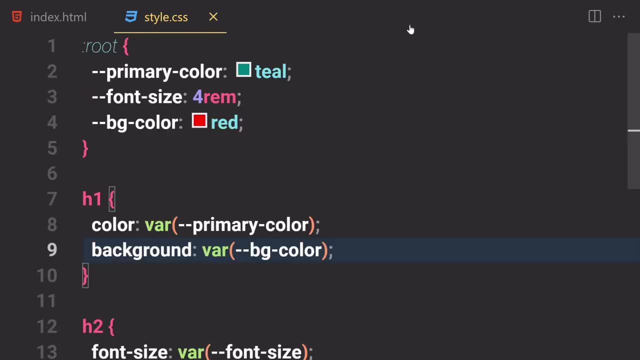 are to just use like bg color for a background. so if you save that and for now change the background color to be totally red and for the change, the heading or the text color to be totally teal, okay, so we can play around with that if you want to. so if i just write white and if you save that, 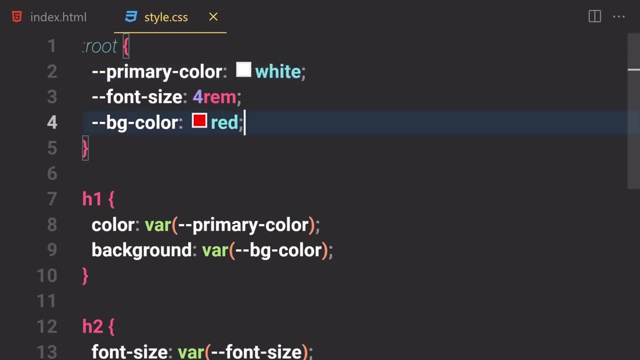 and for now change the color to be totally white. if you want padding, so we can also use a padding. so we just have to use like p or padding you can give like total name. in this case i'm going to just put like p of maybe 20 pixel. and now, if you want to provide a padding of 20 pixel to this, 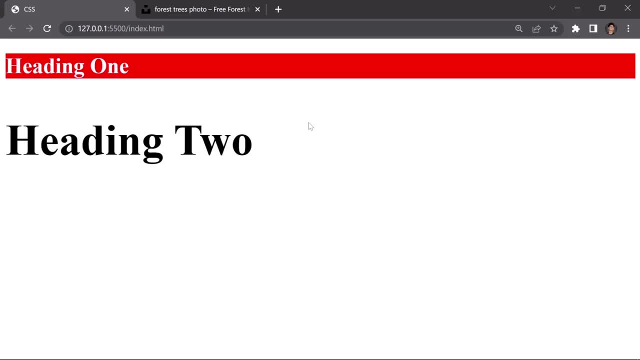 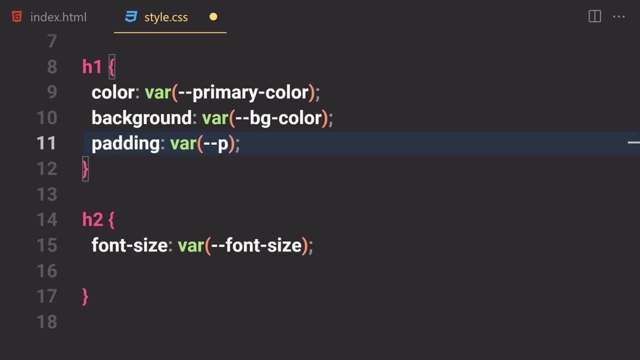 element, so we can just use like padding. or you know what? i'm going to put a padding inside this h1, so i'm going to just use padding, then one and then just a p. okay, two double dashes and p and knife is saved there and it will now just add this padding by using our css custom properties, or you. 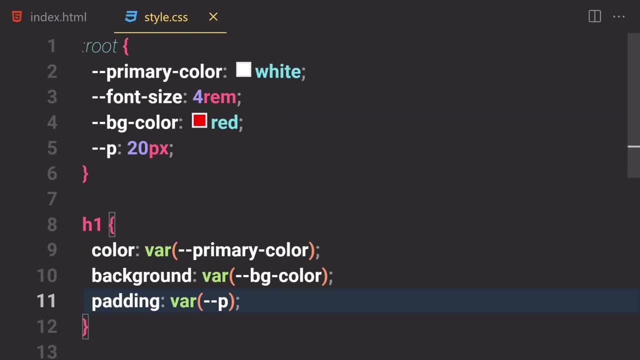 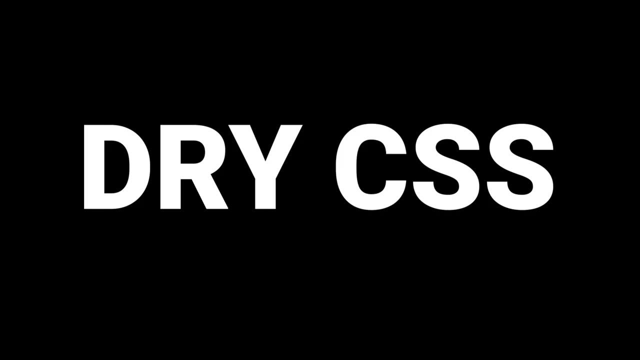 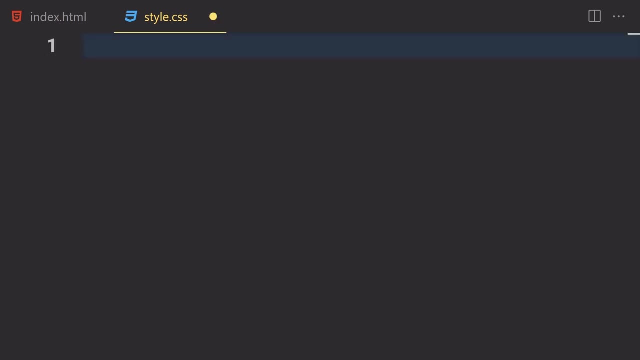 can also call it a css variables. okay, so this is how we can create variable and this is how we can use variable in css. all right, so now that we learned about the css variables, so now the next topic which you are going to be learning about is something called dry principle in programming and in css. 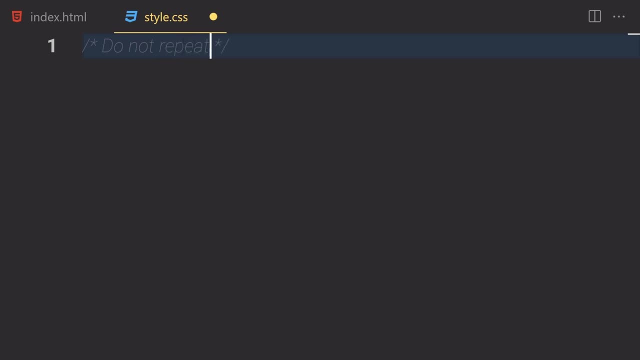 so try, just stand for like do not repeat yourself, okay, so you just have to remember that. and once you jump into like specific programming language, so you will also see this pattern, or uh, what do you want to call it? so you will also see that like do not repeat yourself. 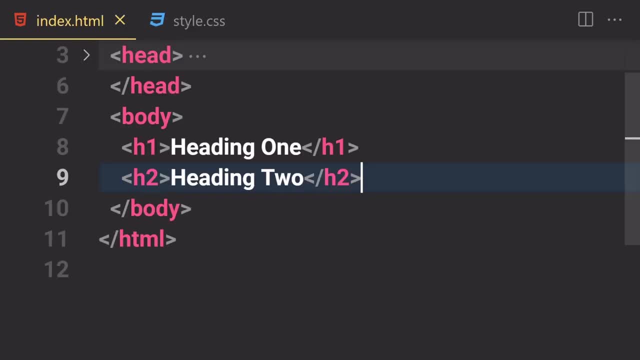 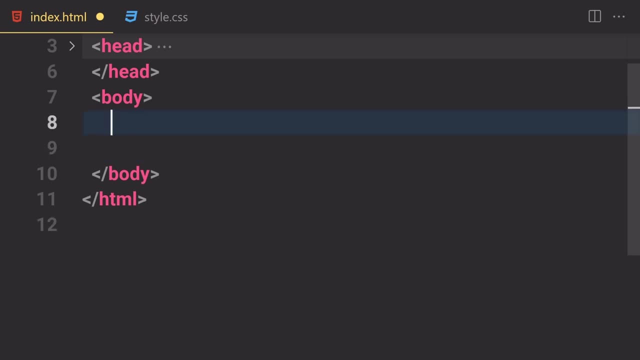 so in css we repeat ourselves a lot. so now i'm going to just give you an example of that real quick. we are going to be first of all writing a bad code and then we are going to be refactoring that code, and, by the way, refactoring just means like we are just improving our code and we are 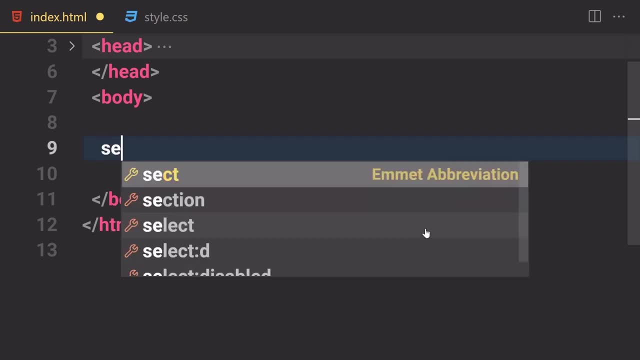 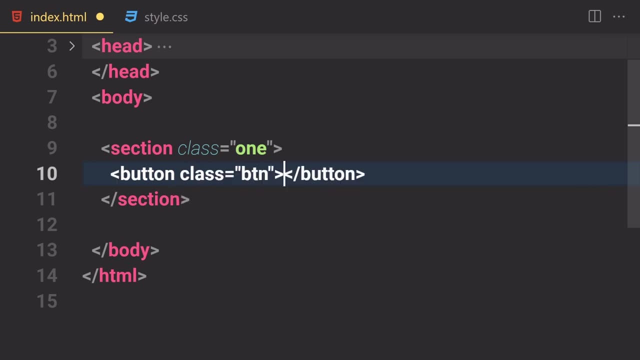 changing our code. so, uh, let's just write a section in here and i'm going to give them a class of one, and now let's just use the buttons, like, uh, maybe the first button someone just used like ptn, of like learn more, okay, and now let's just create a new section right here and now let's just set that. 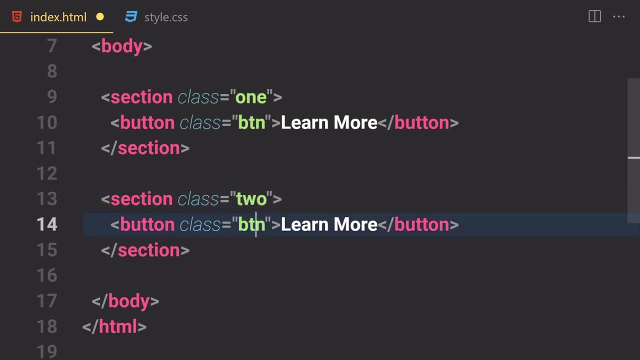 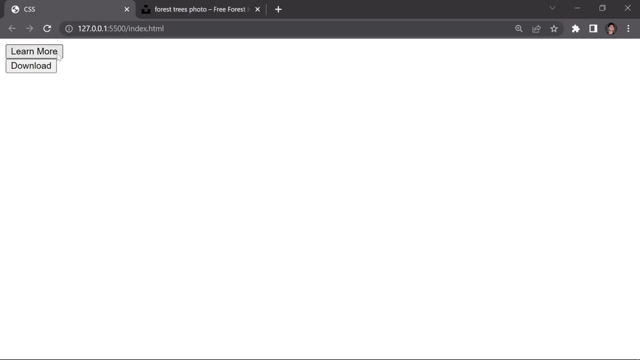 a class to be like two and i want to also provide that btn right there. okay, so instead of learn more, we are going to be just reducing, like download right here. so if you save that, it will not give us two buttons right here, so we just have to put a br in there for not a b. 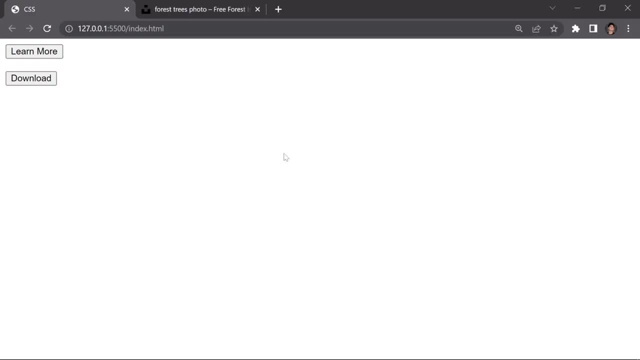 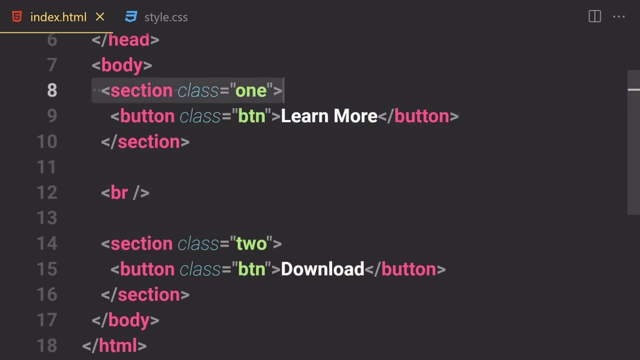 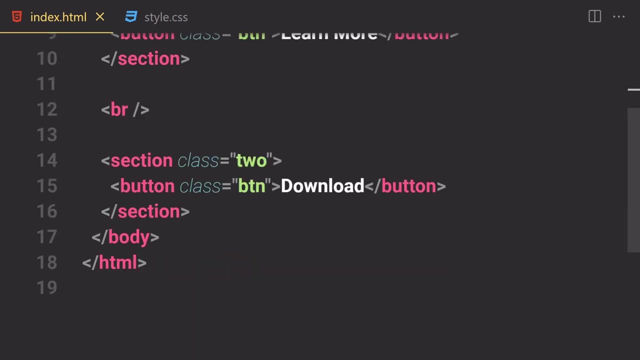 but just a br for a breaking it's like so so you'll not get like breaking in there. so first of all, so here you can see, we have like first section with the class of one and then we have a button inside that section and with the class of btn, and then we have another section with a class of two. 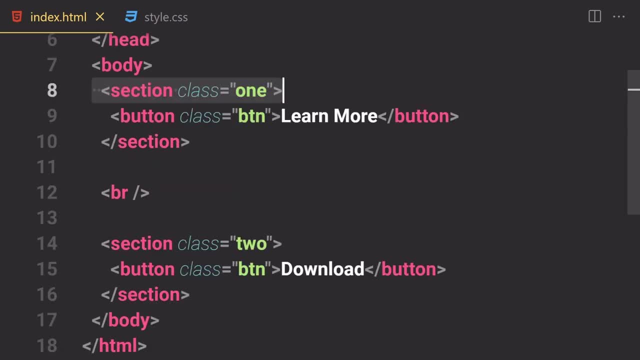 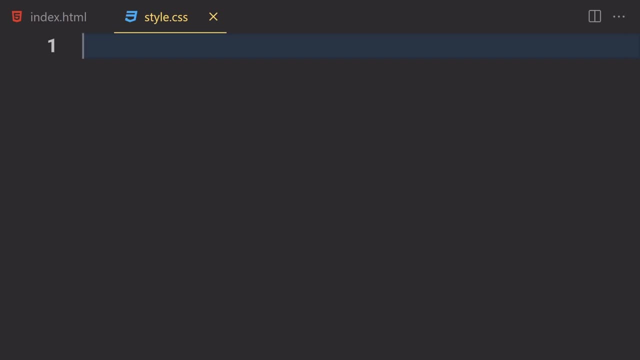 and then we have one button inside there with the class of btn and the title or the level will be just download and this one will be learn more. so this is quite simple and easy. now let's jump into our css. and now, if you want to select that, first of all let me just write a reset form, or you know. 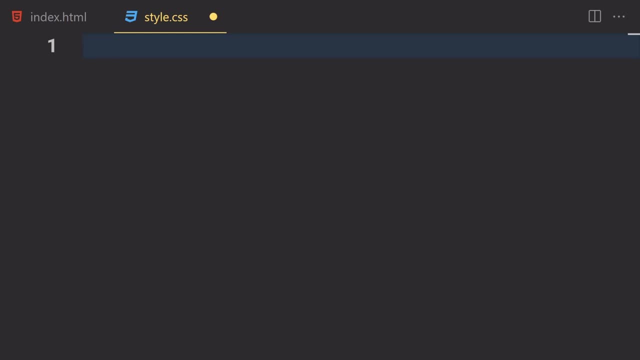 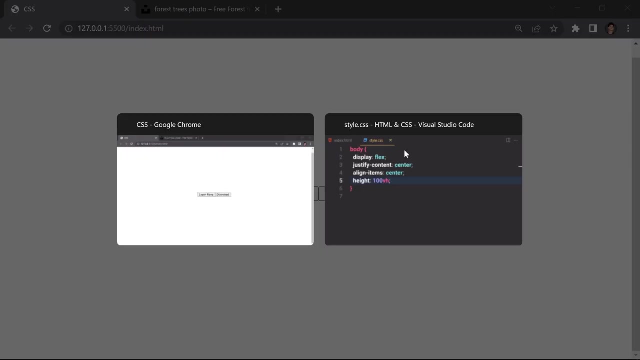 what we will not, or we are not using resetting, so let me just write a body in there, and now let me have flags: justify content: center align. center align- items will be also centered, and i'm gonna also put like 100 vh and save that. and now both of these buttons are now at the center, okay, so let's. 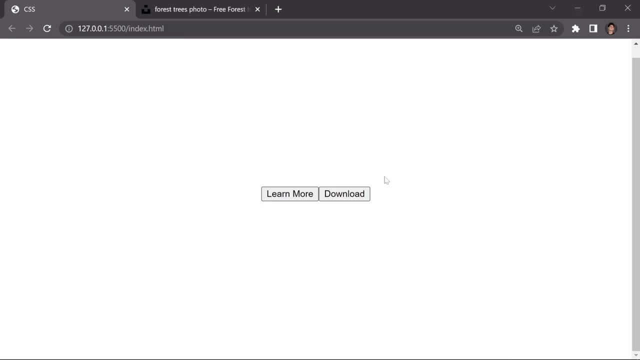 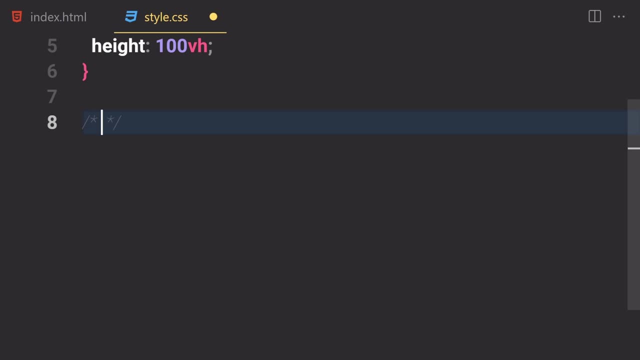 just remove this br from there. yes, all right. so this is it for centering the button. so now, if you want to style each of the buttons. so, first of all, we are going to be using a bad way. someone just write like a bad way of writing. so we are going to first of all selecting the section, then we are. 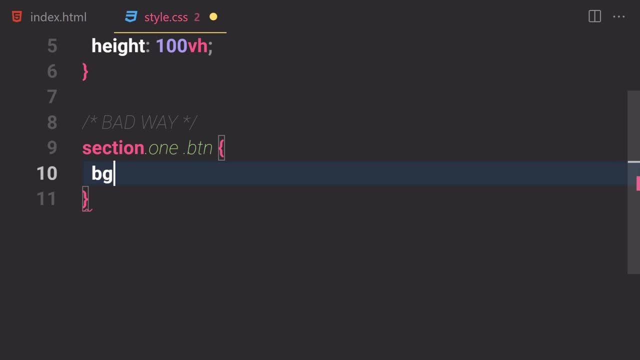 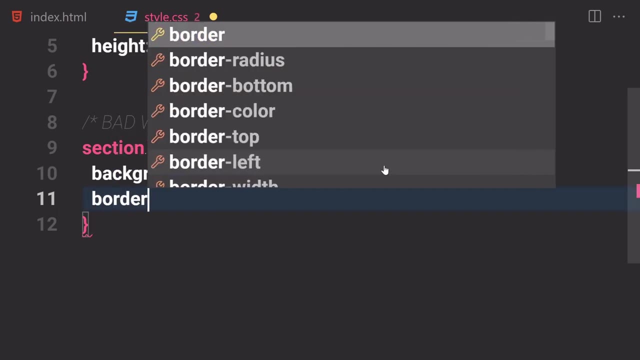 going to be using a bad way of writing. so first of all, we are going to be using a bad way of writing and now we can just use, like, maybe the background of transparent, and we can also use a border to be like none- not border radius, but just a border to be like none. and now we can just use like a margin. 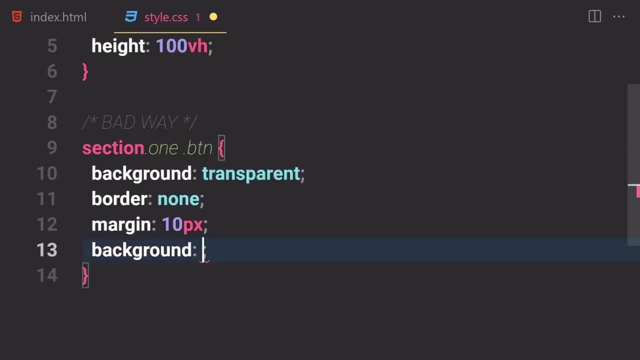 of 10 pixel uh. background will be like: maybe i don't know which kind of color would be fine- rgb of six, uh six. i'm gonna put a six in here one more time. oh my goodness, if i can catch a six. oh my god. so six and six, all right, now let's just put a. 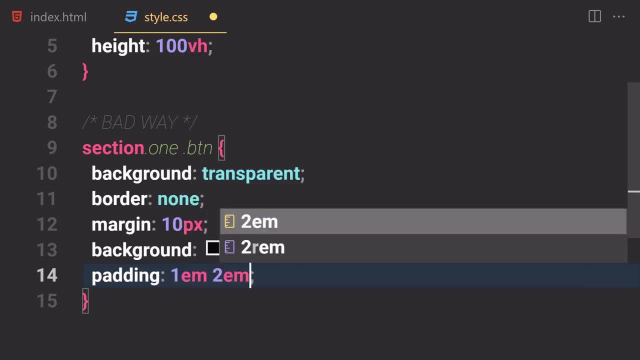 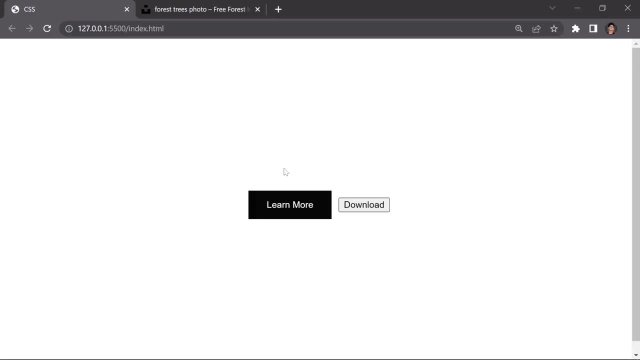 little bit of padding of like one m and two m's, and now let's just give a little bit of color of only white, and also the cursor will be pointer now. if you save that and here you can see, it will now apply all of that styling which i just wrote right here. just release one button right here, like: 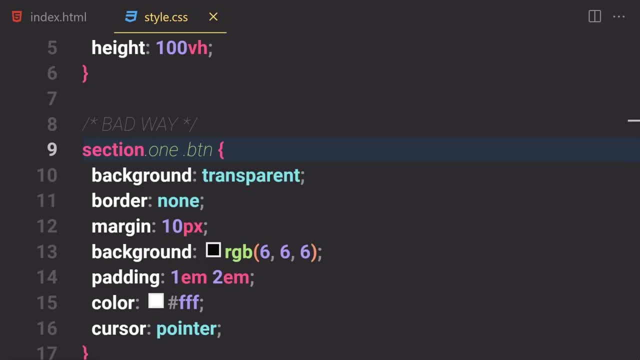 this one btn, class uh, which we specify right here. now we select word section with a class of this one, btn. and now, in this case, if you change the section to be like two and if you save that- so here you can see, it will now apply all of their styles. and now you can see, it will now apply all. 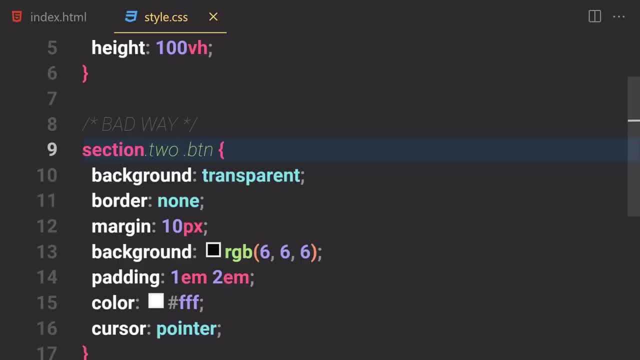 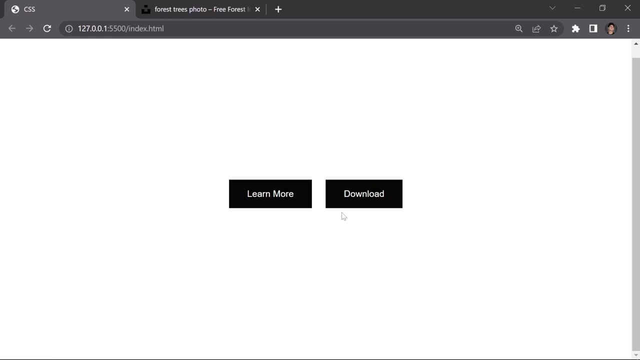 into this button, but not to this one. so we can just remove that first of all. if you just remove that, if you save that, and here you can see, we now solve our first problem. so now, both of these buttons are now taking their styling, which we wrote right here. but the thing is that, if you want, 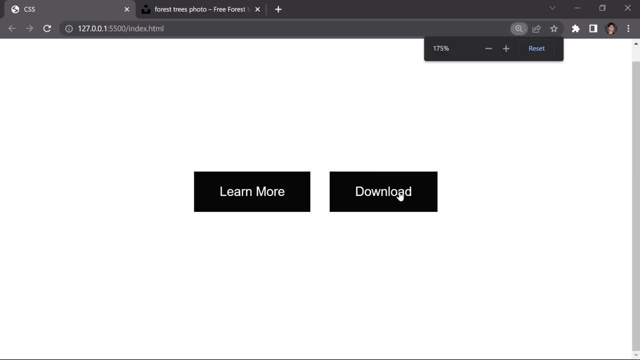 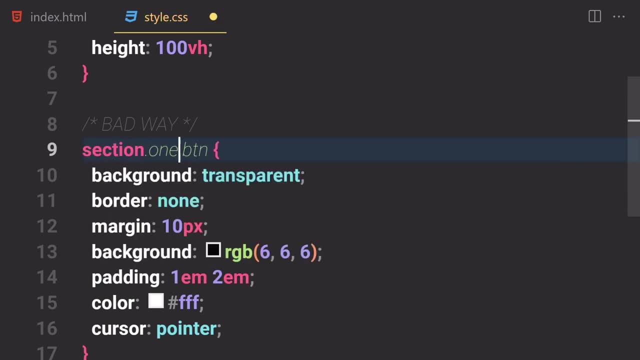 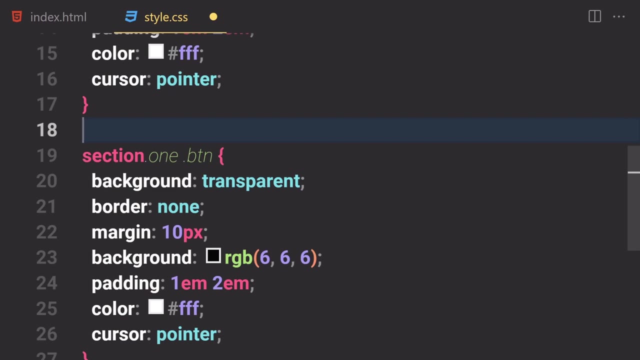 this button to be green, like maybe this download button will be green. so how can we go about doing that? the first and the bad way is that we can just select world section with the class of one, and now let's just duplicate that. so we have just copy all of the content and we will just duplicate that, and now we will just select this. 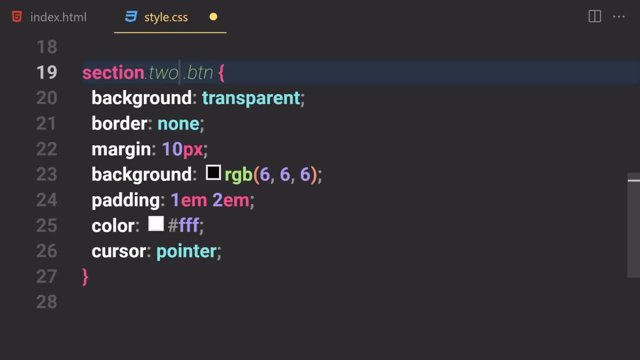 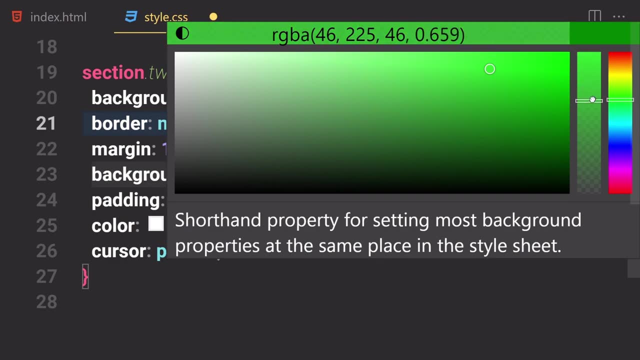 two. um, we will now select this second button and we can just change the color to be like maybe green, and now let's just hold our mouse over to it so you just kind of get kind of a green color, like so, and now, if you sell that here, you can see, now we achieve our result right here. but this is 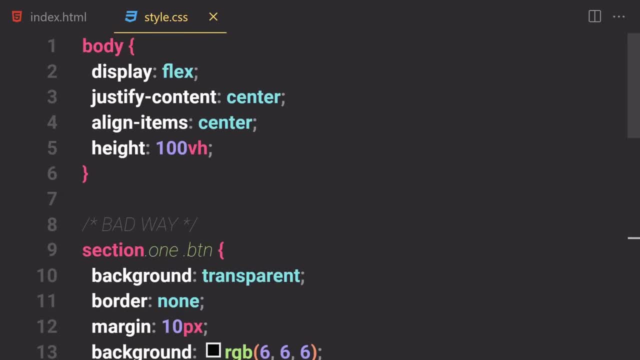 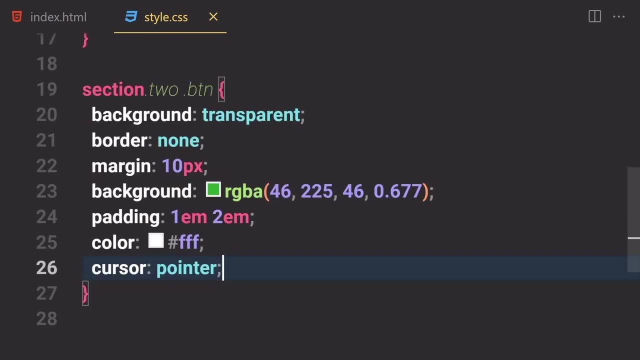 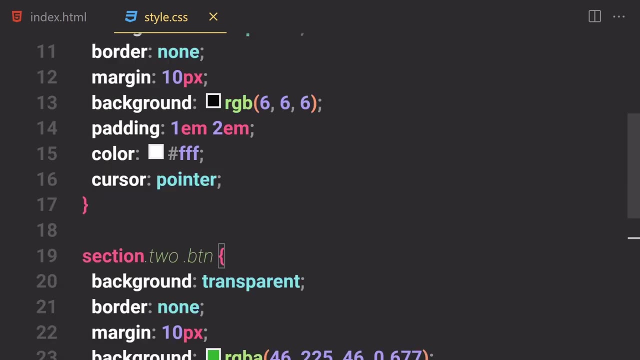 not a better way to write our code, and as we learned in the beginning of the video, is that do not repeat yourself, and this is what a right principle means. so you just found this is just one scenario, but in css you would found yourself countless time repeating yourself. so you just have to think about that principle, like: do not repeat. 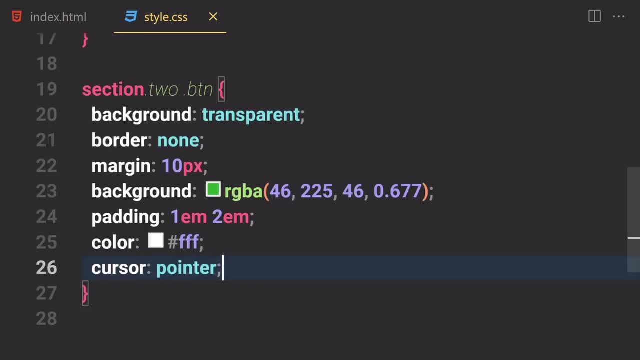 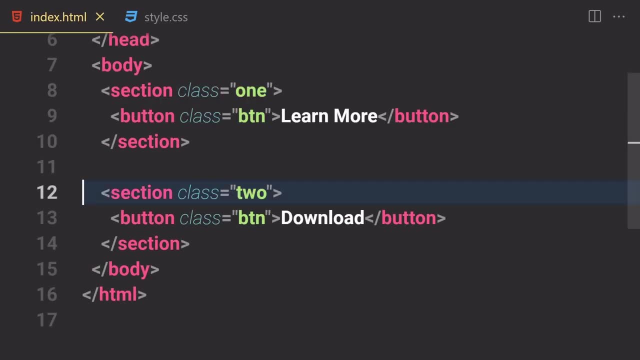 yourself. there has to be a better way. so in this kind of situation, what do we have to do? we can just give them separate clauses to these buttons, so this one will be btn- btn. so now, both of these buttons are now storing all of these styling right here. so now what? 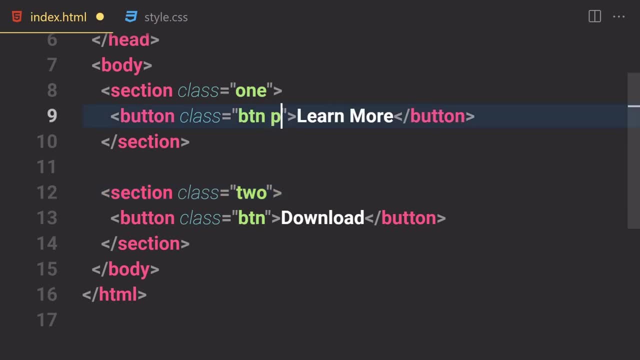 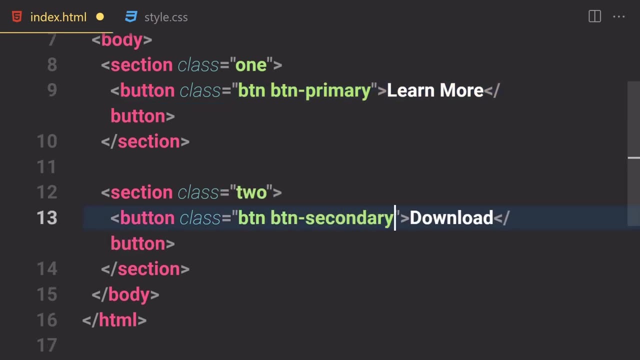 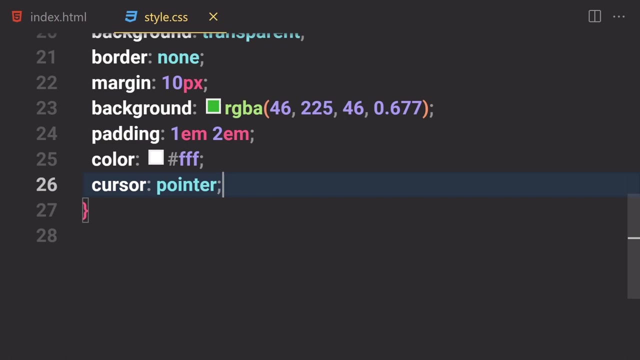 else do we have to do? we have to just give them like new clauses, like maybe btn primary, maybe, and this one will be just btn uh secondary. so now that i give them like a btn primary and btn secondary clauses to it, and now, if you save that, nothing will still happen. so now we 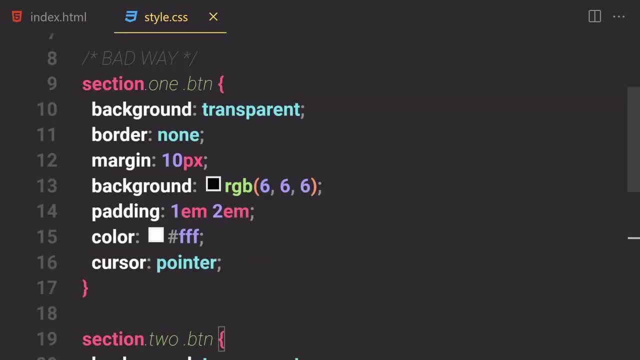 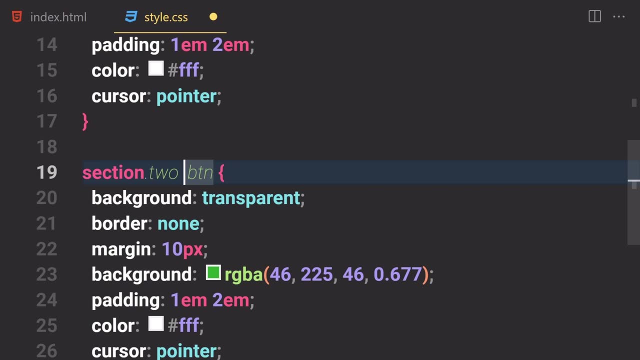 can refactor our code just a little bit- better quality code. so what we have to do, i'm going to just select this section and i'm going to remove that. and now let's just select this section. or you know what? we are not going to be selecting this section, so we are going to be selecting all of. 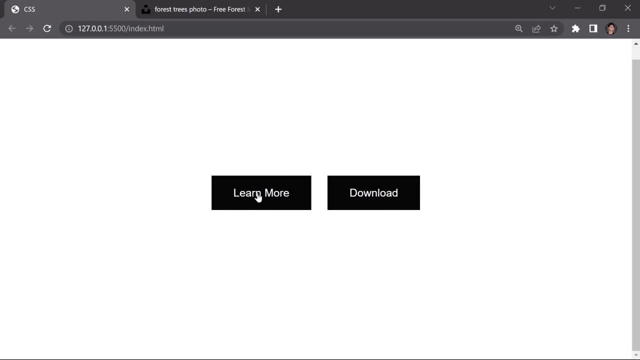 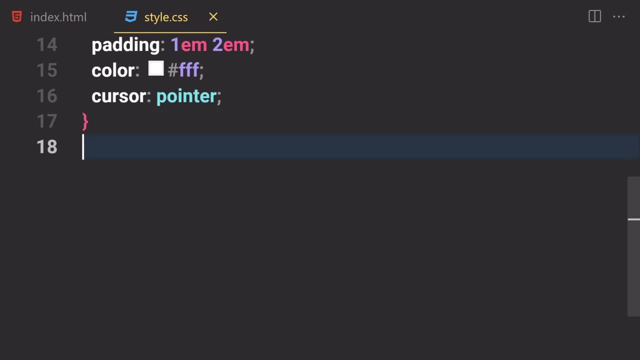 that. so now here you can see that styling are applying to both of these uh buttons right here. but if you want to change the color of this specific button, so for that we can just use uh like maybe a different kind of color, so for that we can first of all use their new class. 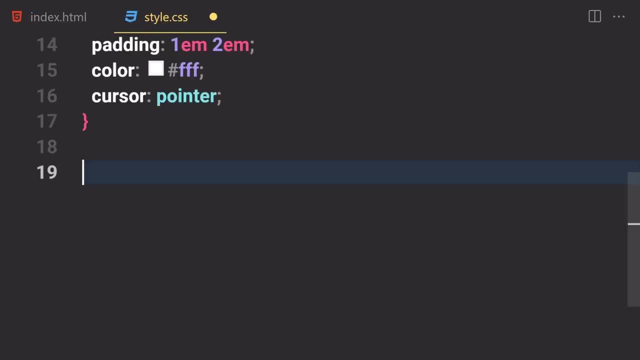 which we provide right here. so we want to select this btn secondary. so now let's just select this very btn secondary. so here we have to just write like a background of maybe green, and now, if you just put a green in there and if you save that, so here you can see, this button is not only green and 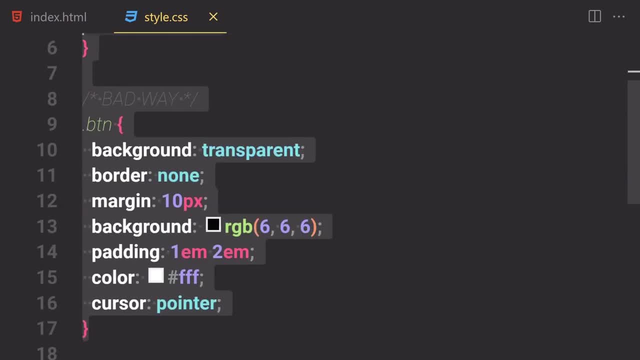 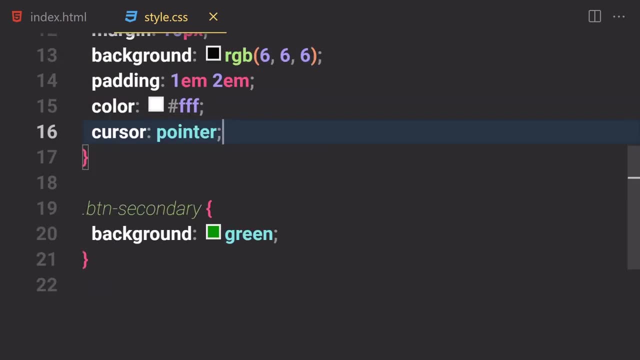 look at our code. we don't have to repeat ourselves, like we don't have to copy all of that code and we have to just tweak things around and we would still have all of these properties and values, but instead of writing all of their clutter code, we now just refactor our code to just this. 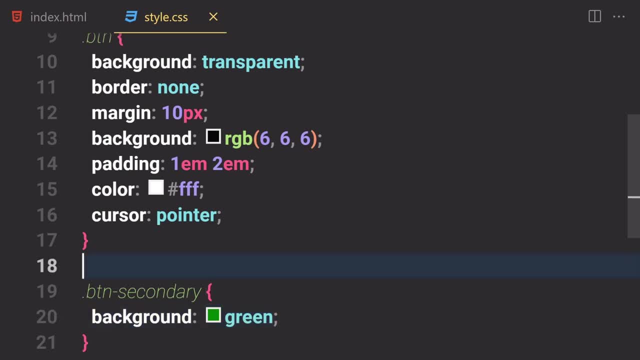 simple one-liner code right here, and i cannot show you all of the ways in this video because it will take a lot of time, but this is just a one scenario in which you just repeat yourself. so so always keep dry principle in your mind, so whenever you are. 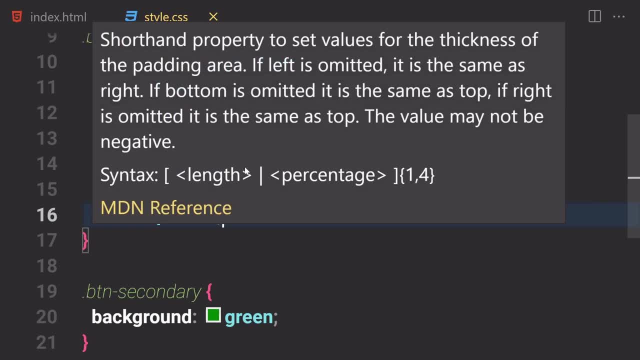 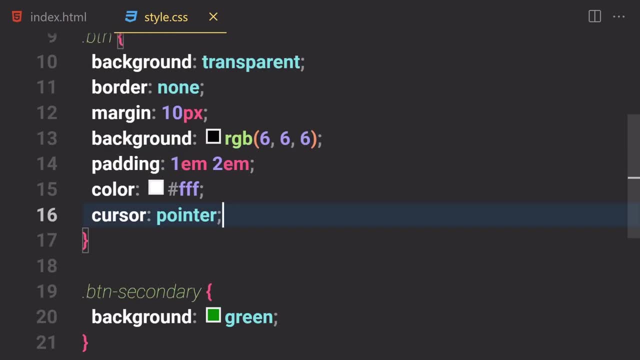 just repeating yourself, or so, whenever you are copying your code from one place to another, or you are just duplicating your code in one or two ways. so you just keep that dry principle in mind, like do not repeat yourself. okay, so there will be situation, you repeat yourself. so i want. 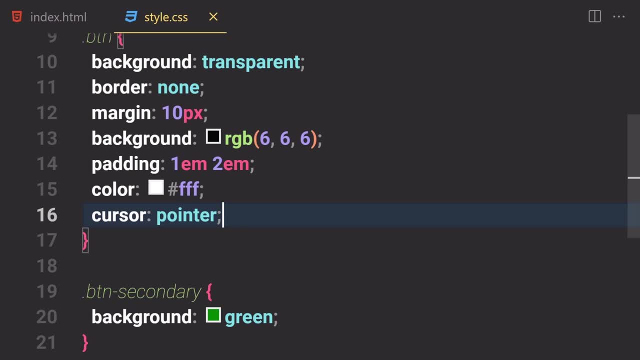 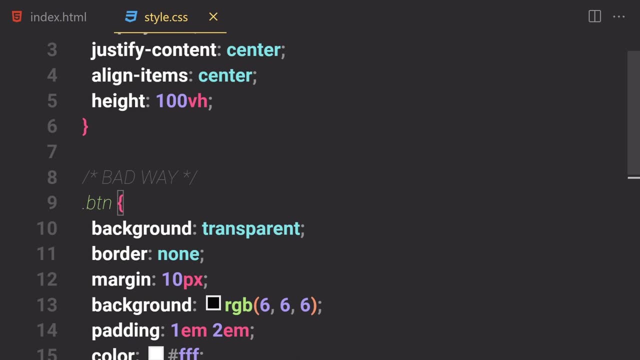 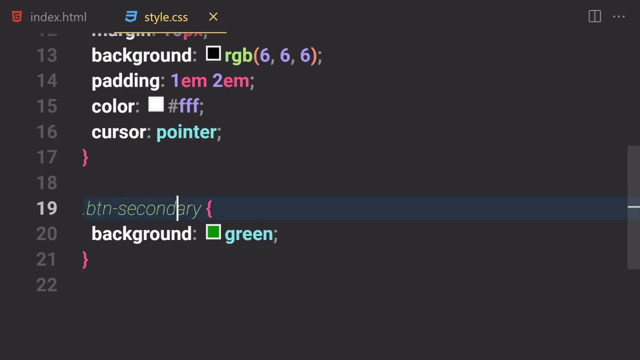 you to just keep in mind this dry principle. and dry just simply stand for like, do not repeat yourself. and there is one more acronym called kiss, and kiss means like: keep it simple, stupid. okay, so we are not going to be learning that, because it's a programming related acronym anyways. so this was at about a dry principle, and now let's get into 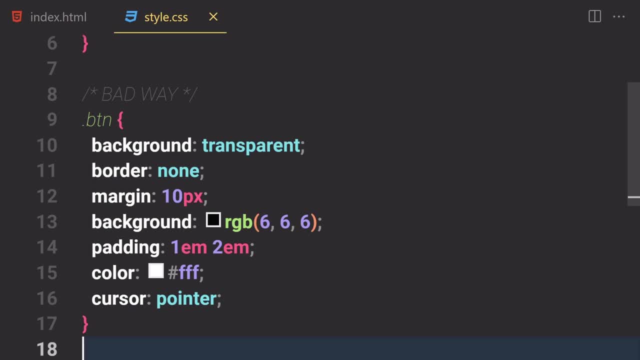 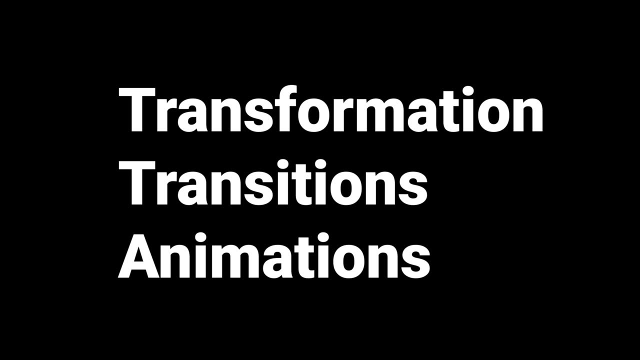 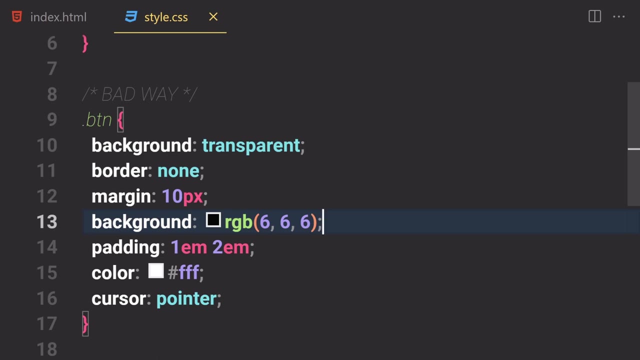 a new section of animation, transformation and rotation and all of these kind of a good stuff. all right, all right. so welcome to a new section. in this section we are going to be learning about transformation, transition and animation. so to learn about that, first of all we have to delete. 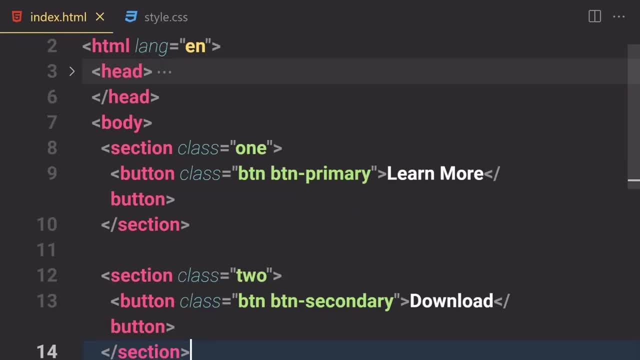 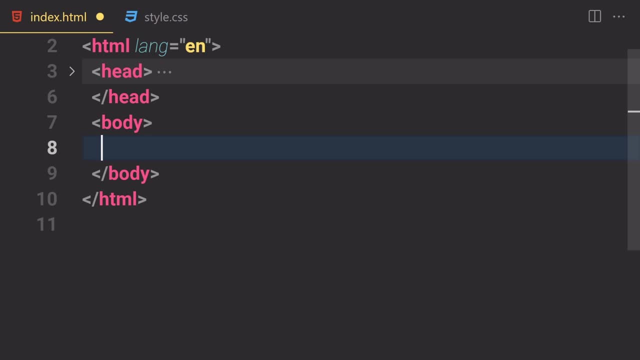 everything which we have inside our style sheet and we are going to be also deleting this section and stuff from our body. so what do we have to do inside our body? and in this specific section, we are going to be first of all starting with a transformation, so we are going to be first of all just writing a section. 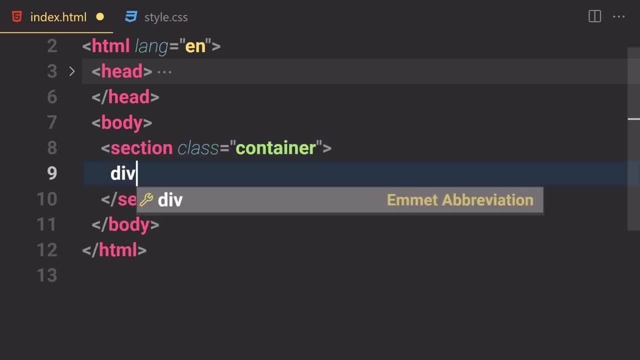 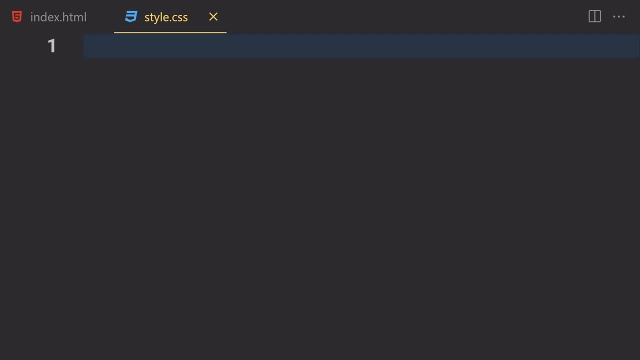 with the class of container. so inside this container we are going to be just writing dev and knife is cell there and go into our style sheet right here. so let's just start working on a transform property. so what is a transform property? a transform property applies a two-term. 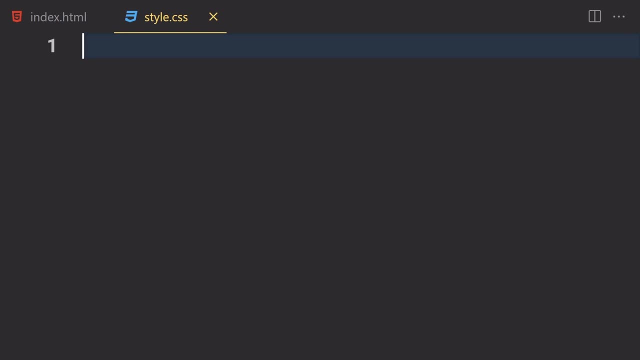 2d or 3d transformation to an element, and this property allows you to rotate, scale, move and scale, which we are going to be learning in this section, just in a second. so, first of all, what do we have to do? first of all, we just have to select our container. we have to give him a height of 100. 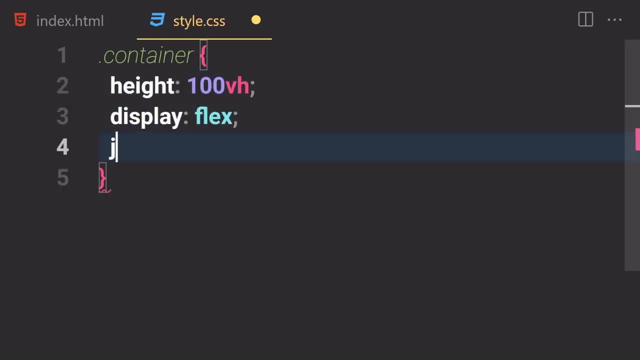 vn so that we can see everything in totally center. so we just have to use display of flags, justify corner of center, align items of uh center. so zoom out, save our file and we can also see something, because we don't have any content and stuff. so now let's just get our container and 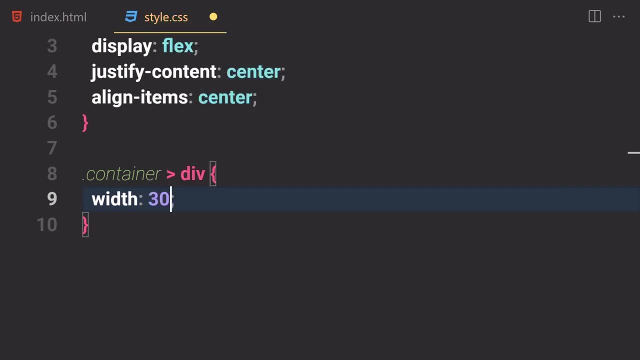 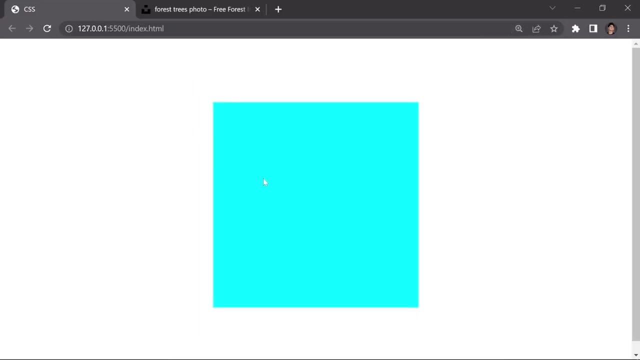 select our div inside that container. now let's just provide a width of like 300 pixel and also the height of 300 pixel. so now let's just give him a background of science or cyan, whatever you want to call it. so if you save that, and now here you can see, we now get totally a rectangle right here. 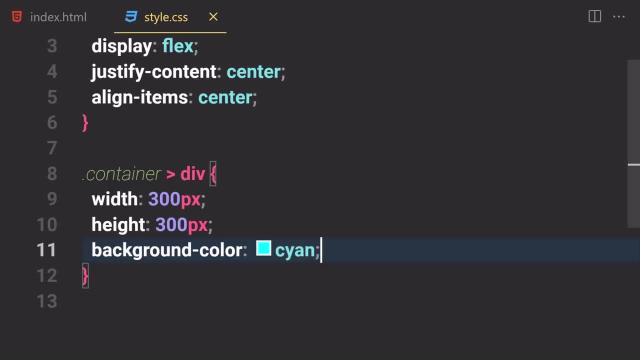 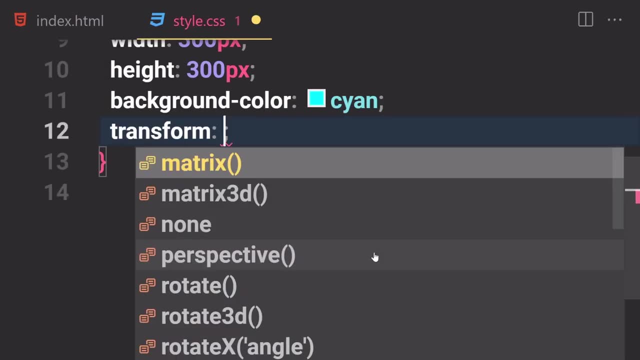 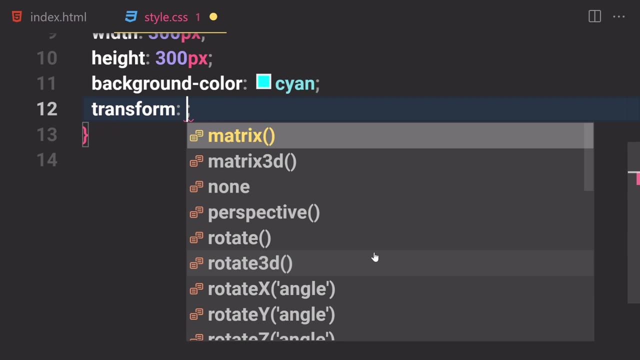 at the middle of our viewport. so now, if you want to transform that, so for that we can use a transform property. so, as the name suggests that it allows us to transform or provide us with a transformation, so now that we use a transform property and we have a lot of values in that transform property, so we are going to be 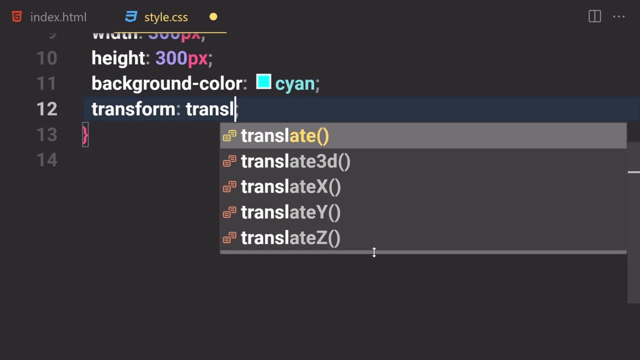 starting from the first one, which is translate. so if you just use like translate or you know we are going to be starting from this translate y function right here and here we have to specify how you want to translate or how you want to move around your element from one place to another on a. 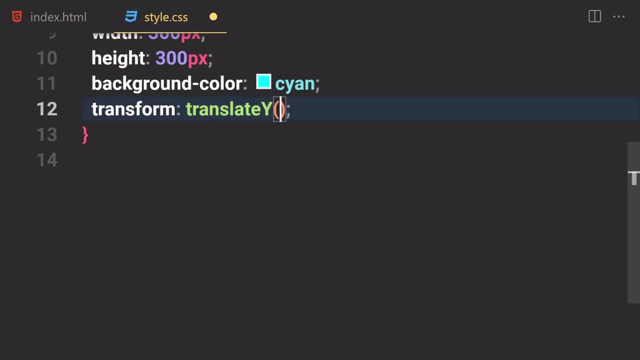 y axis. so now we select for translate y right here. so we just have to specify the amount. so we are going to just, you know, i'm going to just go with like 200 pixel and the 200 pixel will be fine. and now, if you save, 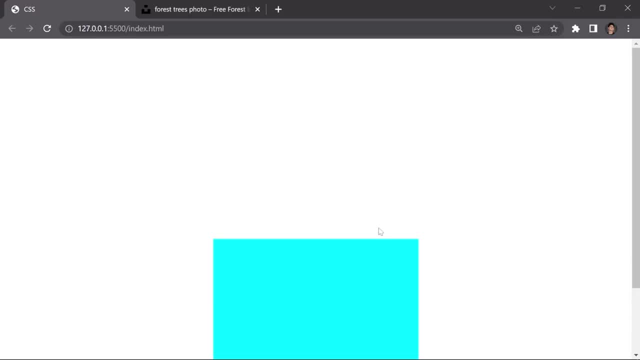 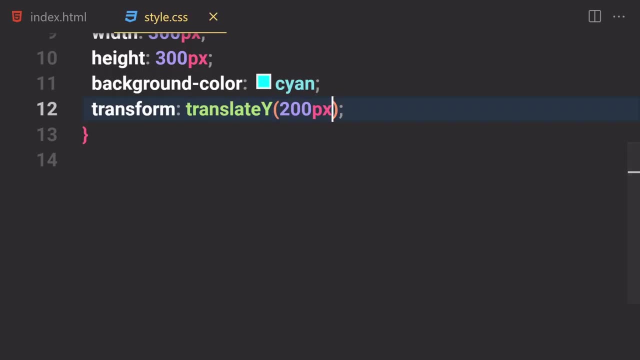 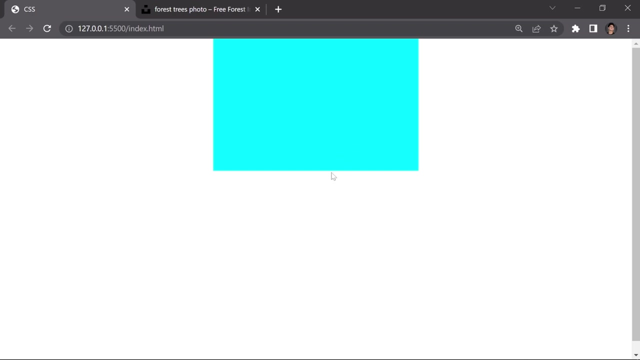 that and boom, so it will now push our container or that box from one place to another. so we just use a positive value, so it will now just push it from top to bottom. but if you just use like negative value, like negative 200 pixel, and now if you save that and boom, it will now push it to the top, right. 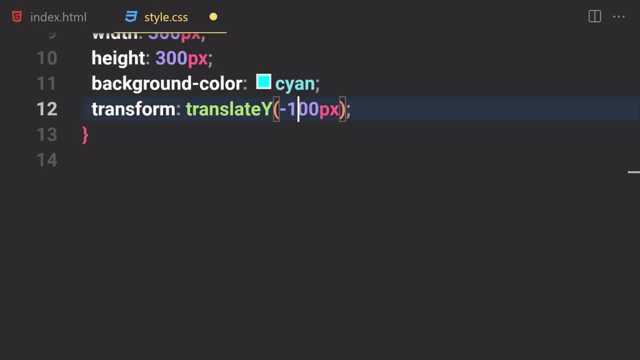 here. so we are not going to be able to do that. so we are going to just use a positive value. so we are limited to just write like 200 pixels. so we can also write like 100 pixel if you want to, and stuff like that. so this is the first value. i'm going to duplicate that and i'm going to comment that line. 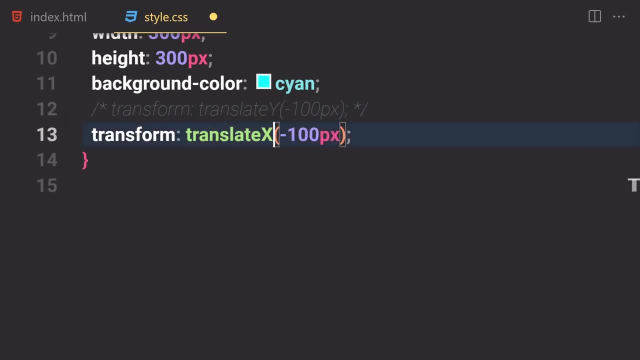 out. and now let's just learn about x axis. so we have translate x. so instead of writing negative value, we would just provide a positive value. but before i show you all of that, let's just comment this line out. and if you save that- and this is how currently, or container, or box, whatever you 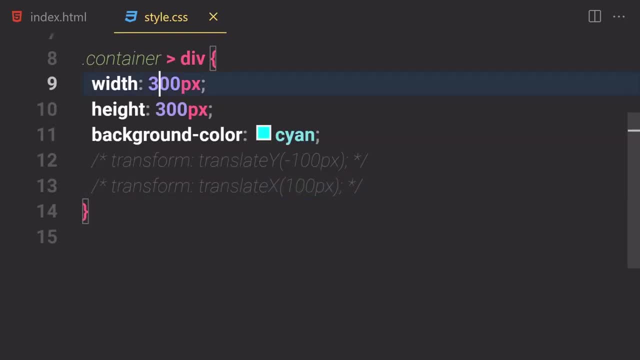 want to call it. this is how it looks like. you know, i'm going to just uh shrink the size to maybe like 200 pixels, so we are going to just write like 200 pixels and then we are going to save it, and that's looking better, all right, so now let me just use this translate: on the x-axis: 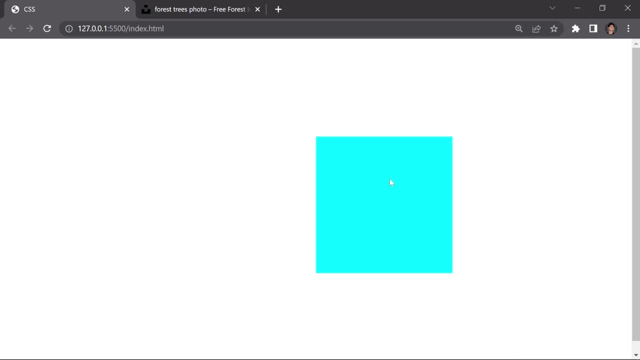 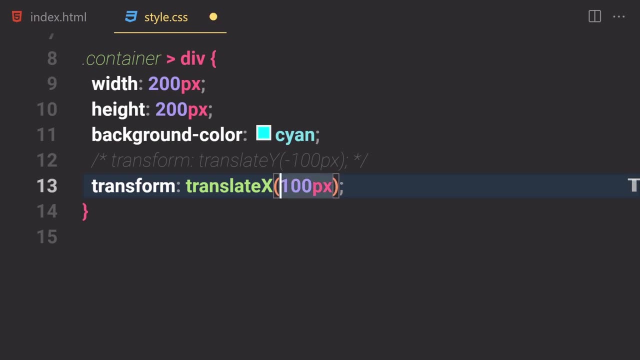 so if you save that, so we'll now just push it to the x-axis like 100 pixel, and we can also just go with 200 if you want to. you can go 300, 000, however you want. so i'm going to just use a negative value. 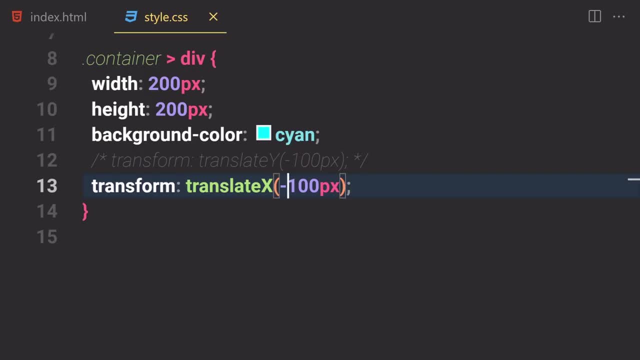 in this case. so if you save that and boom, it will now push it to the negative 100 pixels. so if you just use like negative 200 pixel, so we'll just push it around by using this uh transform of translate x-axis and translate y-axis. so now let me just comment this line out. 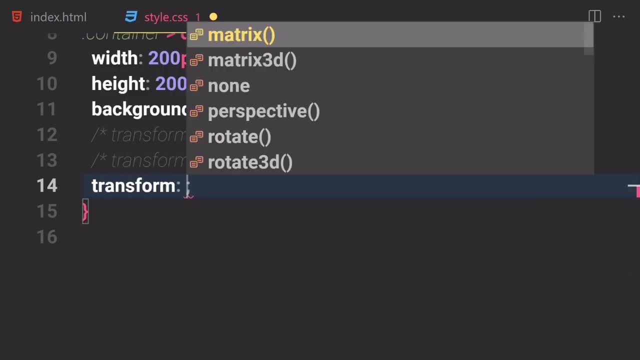 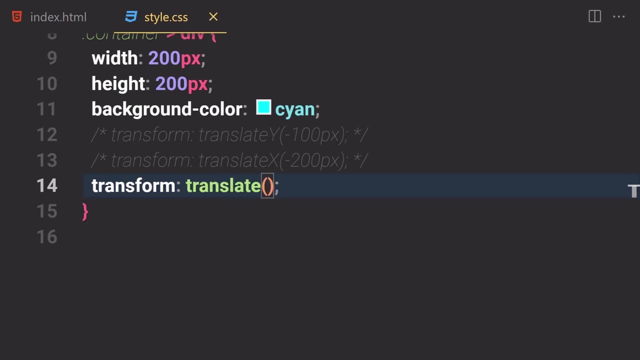 now let's just use that transform same property. but instead of translate x and translate y, we can just use a translate function right here and now. the first value which you have to provide for the x-axis. so we are going to be providing a value for the x-axis like 100 pixel, and then we have to put: 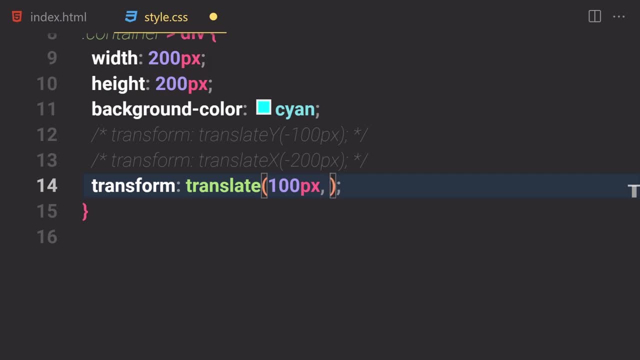 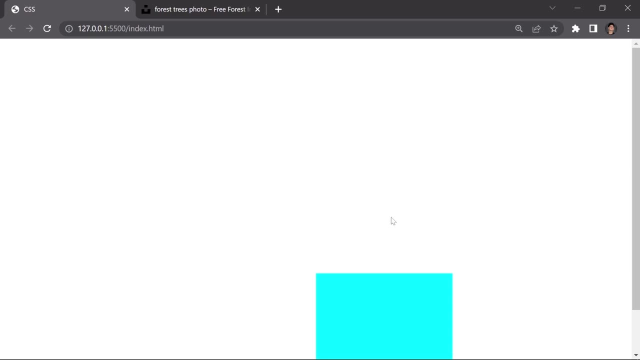 a comma in there and then we have to specify the value for the y-axis. so i'm going to just put like 200 pixels, if you save that, and it will now push our item from left to the right like 100 pixel and from the top to the bottom like 200 pixels. so we can also use- uh, you know what i'm going to just. 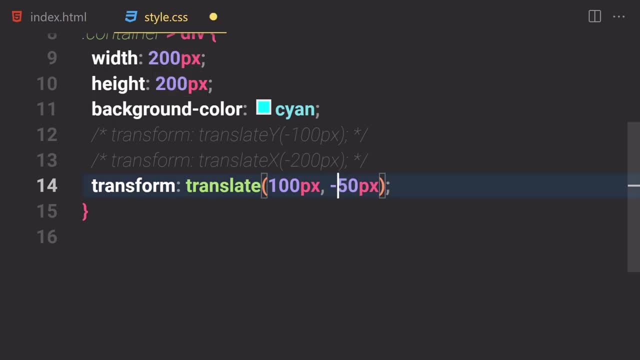 push it to the 50 and we can use a negative value for that. and if you save that, so we'll now just push it a little bit. if you just use a positive value, so we'll just push it from top to bottom. if you just use a negative value, so it will now push it from left to right. 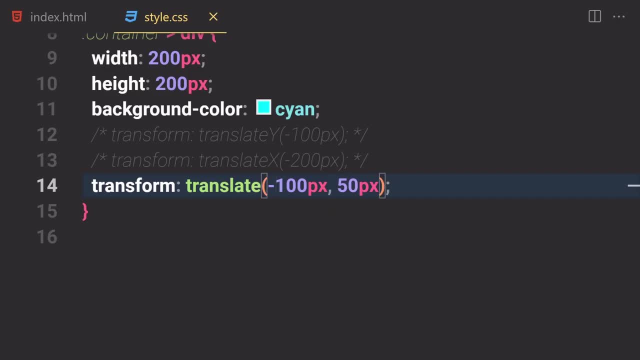 like so, and you can play around with this property if you want to. i'm going to comment this line out now. the next value which you are going to be learning about inside this transform property is a rotation, and this rotate property will allows us to rotate over elements. so, in this case, what do we have to do? we have to just specify the rotation. how? 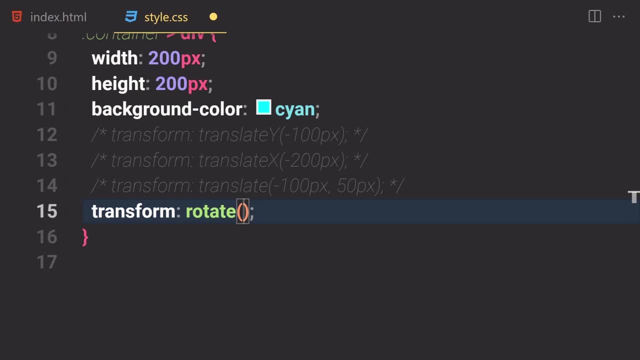 many rotation we want. so in this case i'm going to just provide like 20 and d, e, g for degrees. so if you save that, it will now just rotate or element on a 20 degrees so we can provide more degrees. if you want to like 40 degrees and boom, it will now just rotate it on a 40 degree. 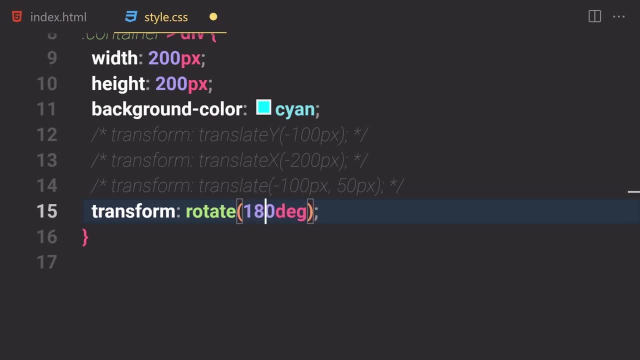 so if you just specify 180 degrees and save that, so you just get a default result right here and we can play around with that, like maybe- i don't know- 60 degrees, and this is how it looks like. we can just move it to like 10 degrees, 20 degrees, 40 degrees, how many you want. okay, so this rotate. 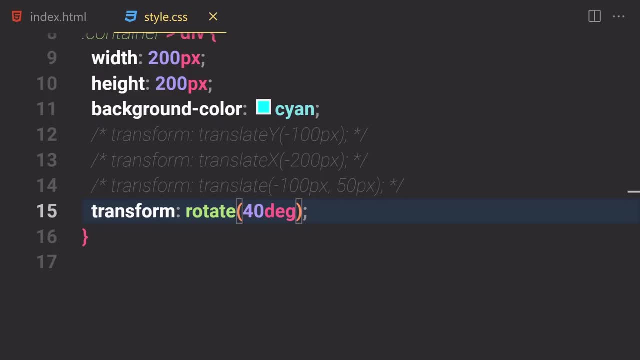 function will allows us to rotate over element. i'm going to comment this line out as well. and now let's just use a transform of scale, and this one is my favorite one. and as an example, i'm going to just use a transform of scale, and this one is my favorite one. and as an example, i'm going to use a. 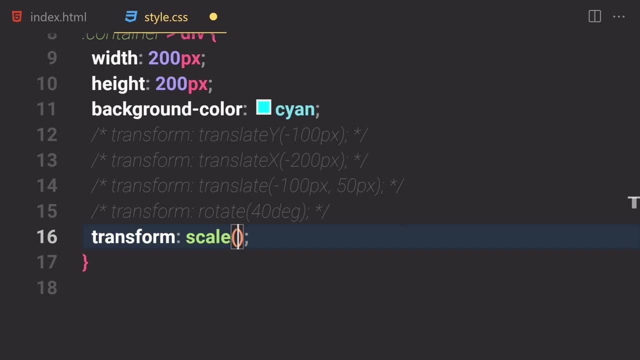 transform of scale, and this one is my favorite one and as an example i'm going to use a transform. it will slow a little bit and it's going to show that 20 degrees and it got really high. ok, now, like i just discovered, only сотрудka, like for this law, and i got all that for only. 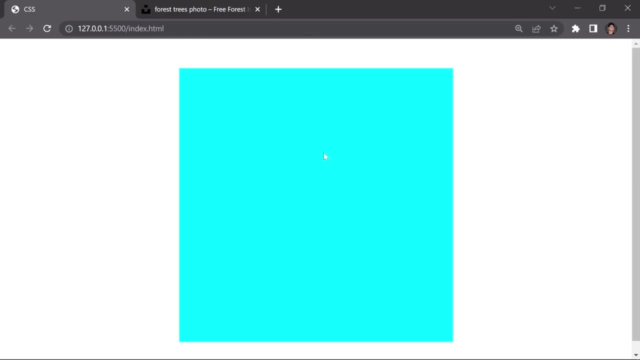 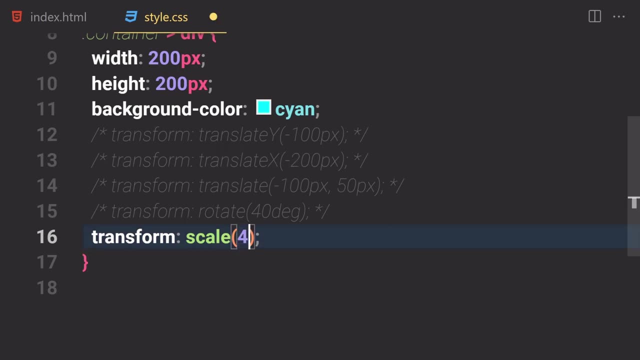 just initially. and okay now if we just scale it to like that. so first of all, let me just, and so it will now just scale or element on two. so if you just write like maybe four and if you save that and boom, okay, so it will now scale it like four time of the current size. so we can just 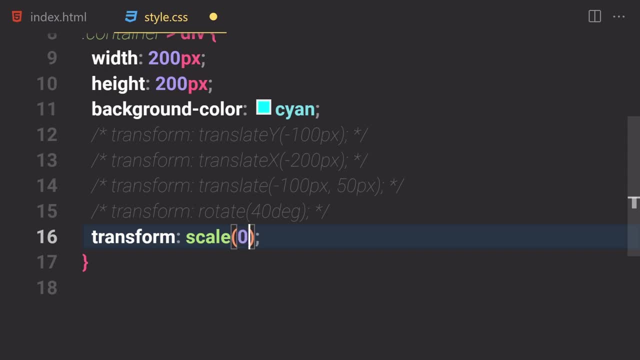 use like one, or we can also just decrease that, if you want to. so we can use like 0.5 and save that and boom, it will now just decrease it to 0.2 and it will now decrease it however we want. so it's. 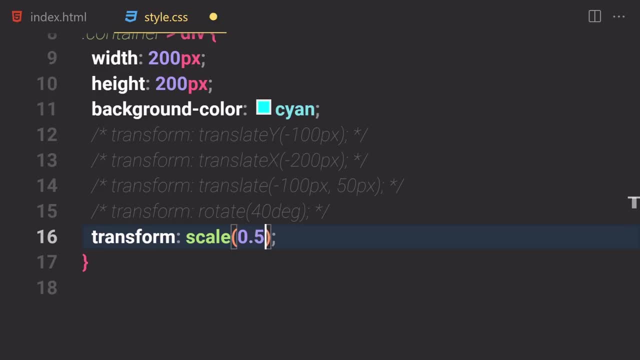 kind of like a smaller container box right there, and this is how we can increase or decrease our element by using our transform of scale value, and we can also provide a value for x-axis and y-axis. so now let's just put over five in their bag and if you just put a comma, and if you put one and 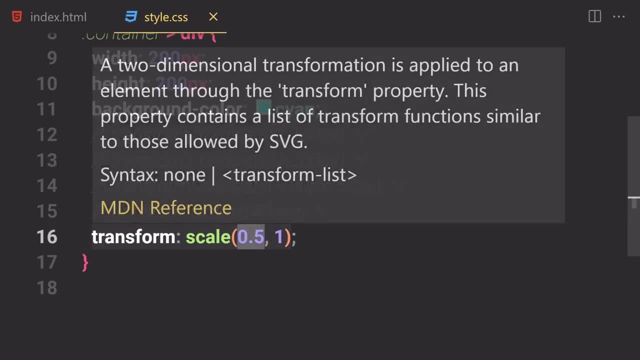 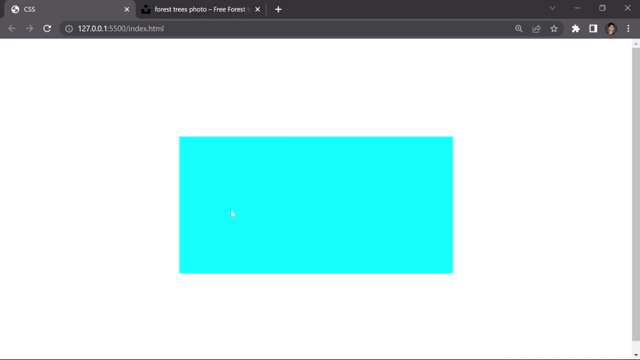 save that, so this value will be for the x-axis and this value will be for the y-axis. so anything we put inside there, like two, and if you save that, so it will just increase the size of the x-axis. if you just set this one to two and if you save that, so it will now just increase the size. 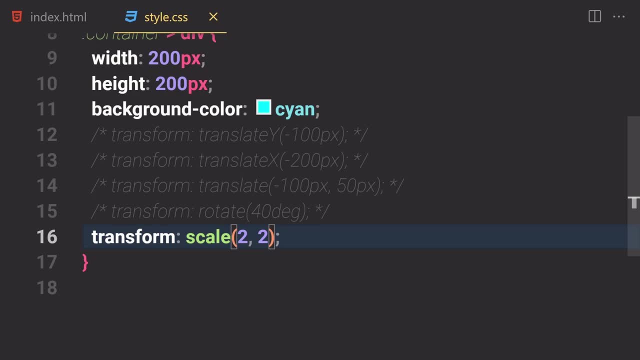 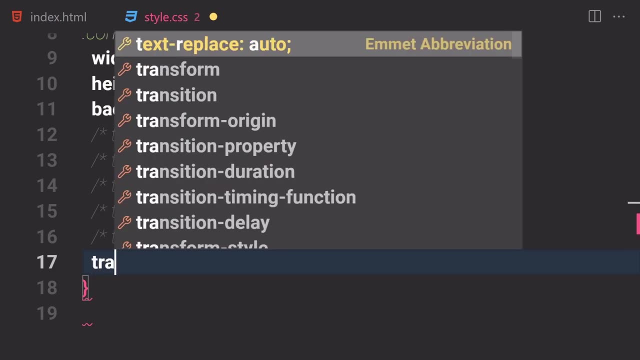 of the height, like on the y-axis. so this is how you can play around with that if you want to, and i just show you that. so now, the next value which you are going to be learning about is something called a skew, and we'll just kind of, uh, tell tech, put that in words like a skew. what is it you want to skew? 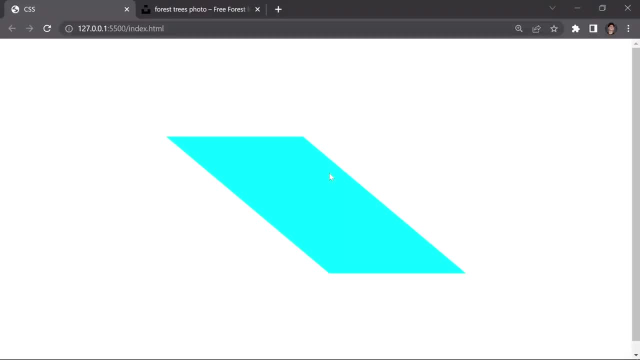 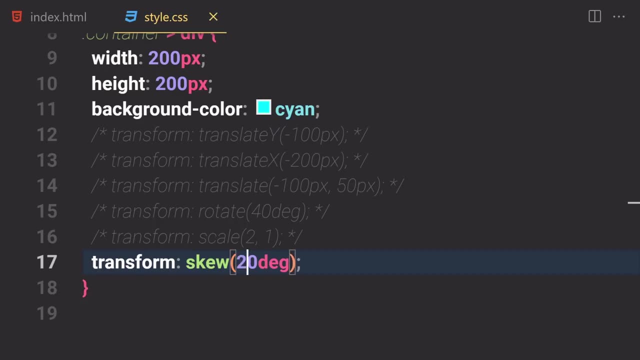 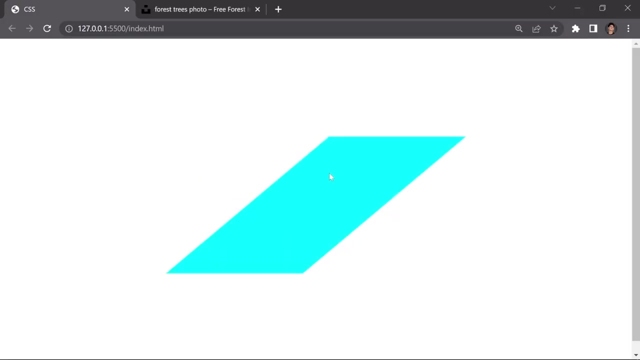 so you can just pass four degrees in there and if you save that, so we'll just skew it up like so: if you just put like maybe 20 value, and we'll just skew it with the x-axis and we can also put our y-axis if you just save that. so this for x-axis we can just use like negative value and 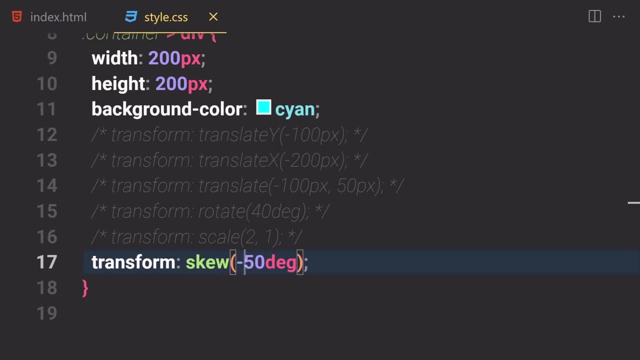 now just totally convert the shape of that. so this is how we can use a transform property, and transform property can do more than that. but this is just an introduction of that. so in this section we just learn about a transform property and its different values. so we learn about translate y. 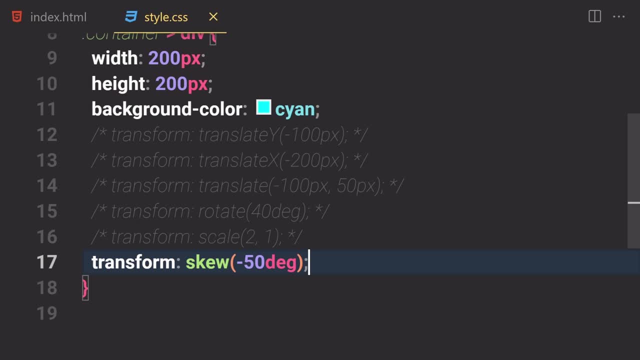 translate, x translate and rotate, scale and skew. okay, so i guess that would be it for this section about a transformation, and now let's just learn about transition in css. so for that, i'm going to remove everything from my container, and i want to also remove these heights and widths, or you know, i'm 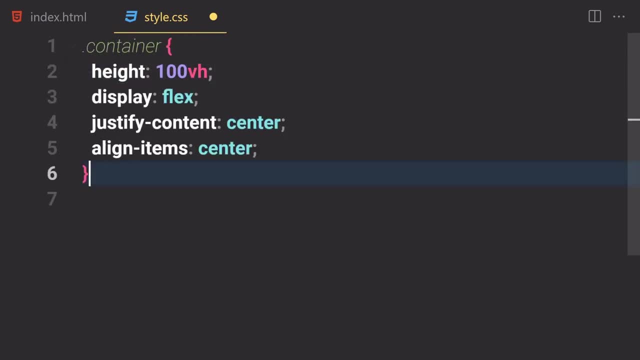 going to delete this container. just leave this height and display of flex and stuff. i'm going to go to my html and i want to change this div from div to anchor tag. it will go to nowhere and it will just say like, click me and if you save there and we will just get or click me button at the 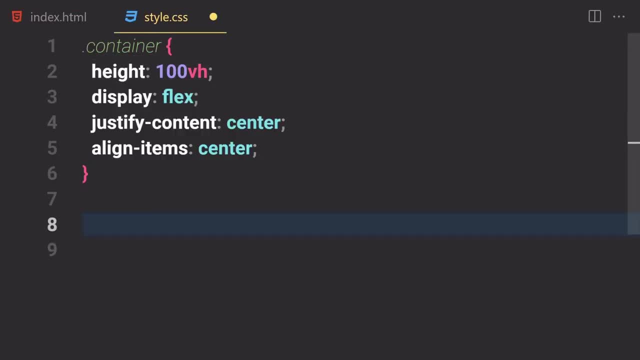 center of our viewport. so now let's just start working on our container. so first of all, let me just select my container and inside that container we are going to be selecting our anchor tag. and now let's just remove their text decoration of none. okay, not text align. 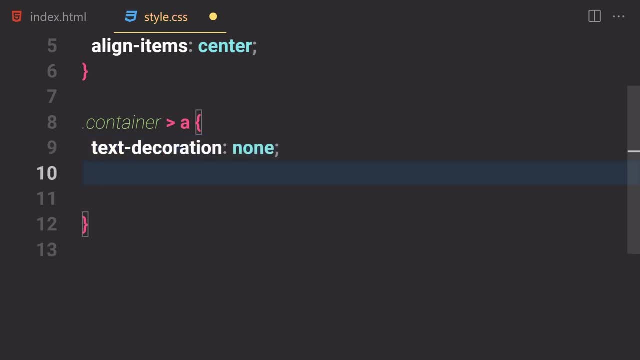 but text decoration of none. now let me just provide a border of two pixel- uh, solid, totally red. and i'm going to also provide a padding of 10 pixel and 20 pixel. 10 pixel for the top and bottom, 20 pixel for the left and right. color will be totally brown, uh, brown. and now let's just go to. 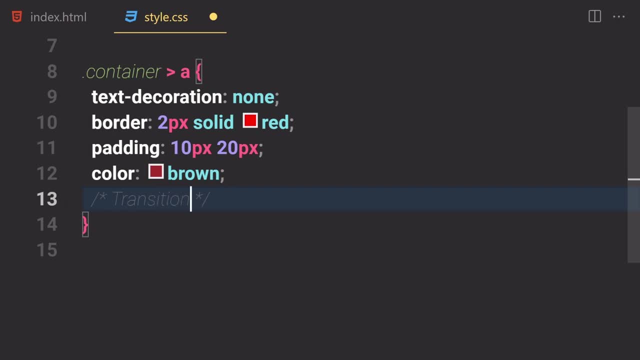 transition and let's just work on our transitioning. so transition, i guess i spelled it correctly. so what in the world is even a transition? even mean. so css transition allow you to change property value smoothly or a given duration. so you have to specify some sort of a duration so we can change. 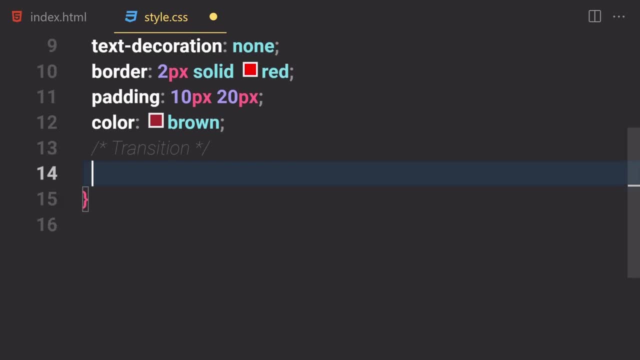 whatever you want, totally smoothly. so i'm going to just show you that and then you'll get to know what is that transitioning you would mean. so now, if you want to work with a transition, first of all we have to change something. so let's just go to transition, and let's just go to transition and let's. 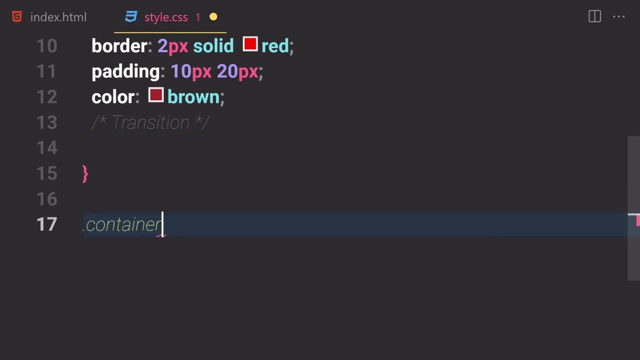 change something. so if you want to change something, so for that we can work with or hover, uh, pseudo selector, as we learned at the beginning of the video. so if you just write like anchor tag and hover, and now let's just use like a bg of color and maybe it will be set to like brown. 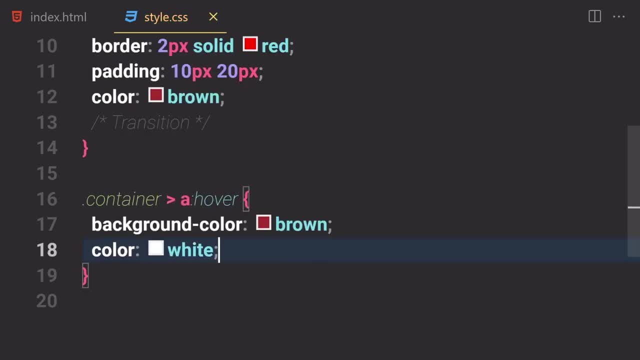 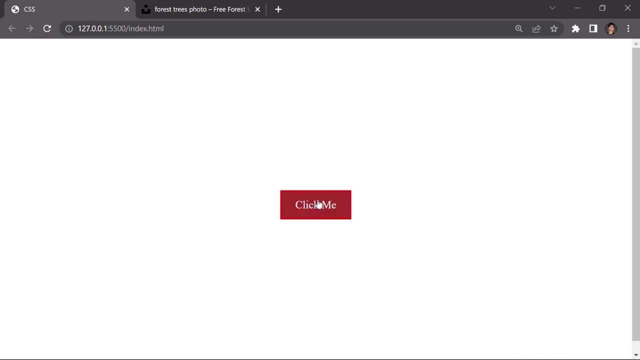 in this case and now let's just provide a color of only white. so if you save that, and now if i hover my mouse over to it, so here you can see, it's now changing its color very quickly right here. so if i hold my mouse over here, so it's now changing this color in a second or maybe a half of a second. 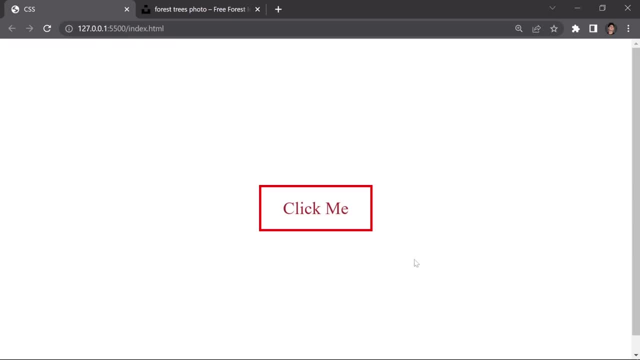 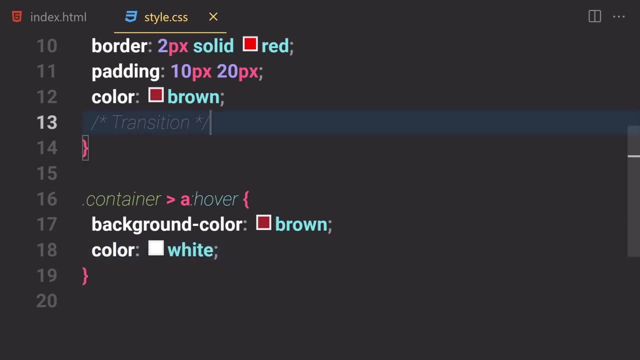 stuff like that. so if you want a little bit of transition to happen, like if i hover my mouse over to it, so we want a little bit of delay in there, so we can do that by using our transition property. so now let's just start working on our transition property, so for that we can just use 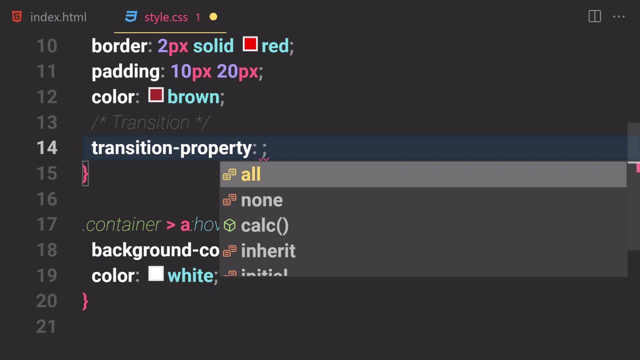 our transition property. like a transition property simply means like: what do you want to change? okay, so we want to change everything. so now, in this case, it will accept this background color property and also this color property. so if you just provide like border radius or any other property, so it will also accept that. and if you want to accept like a specific. 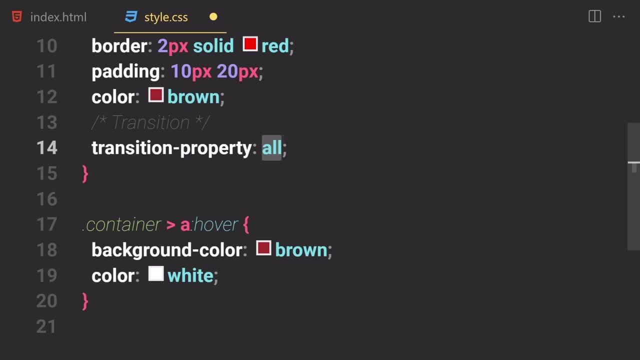 thing. so for that you can just provide the name of the property. in this case, if i just retry like background color, so we can also work with that. so if you want our transition to just only happen for a color, so we can also specify a color. so now, in this case i'm going to put 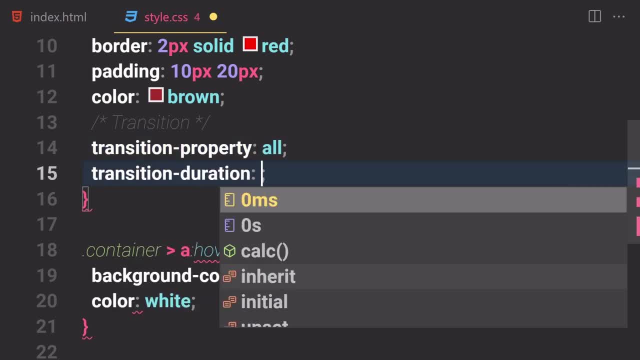 everything to all. and now the next thing which you are going to be learning about is something called transition duration property and, as the name suggests, that it will just wait for that much duration we provide right there. so let's just wait for that much duration we provide right there. 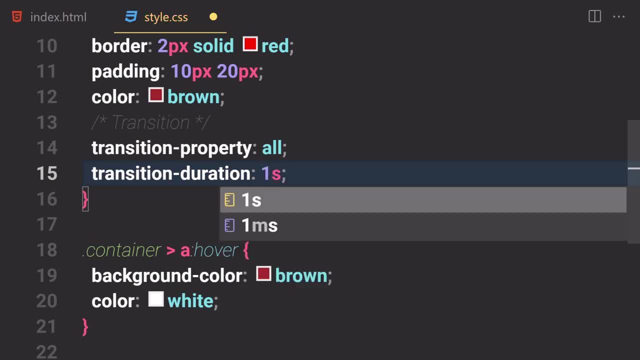 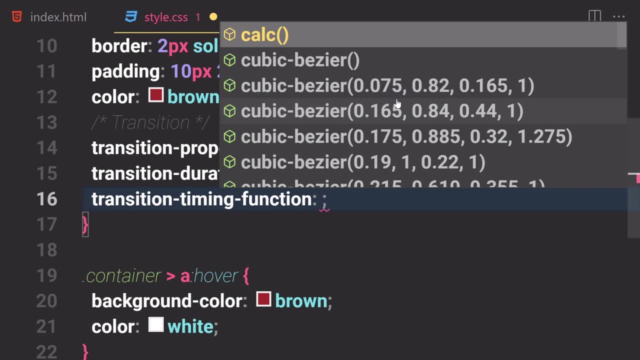 so in this case, we are going to be using like one second. and now, finally, we are going to be using another property called transition timing function. i know this property is a little bit long, but there are a lot of transition timing function out there, but in this specific video we are going to be 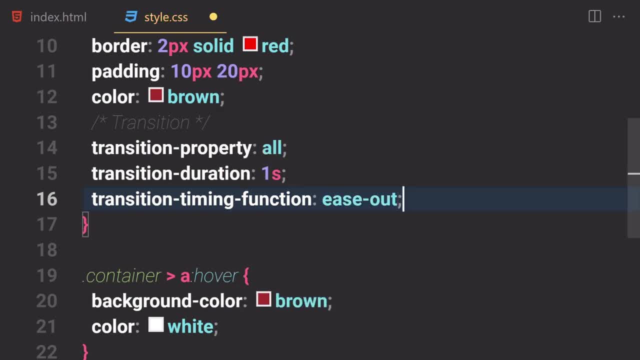 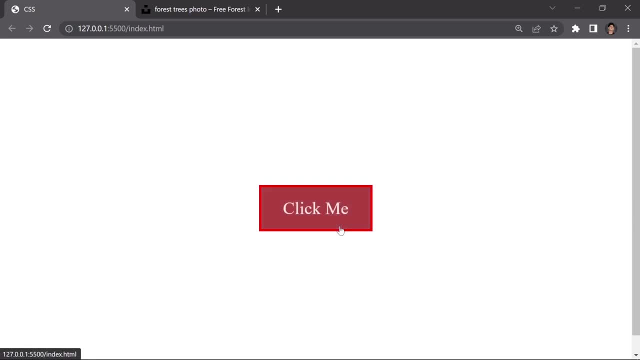 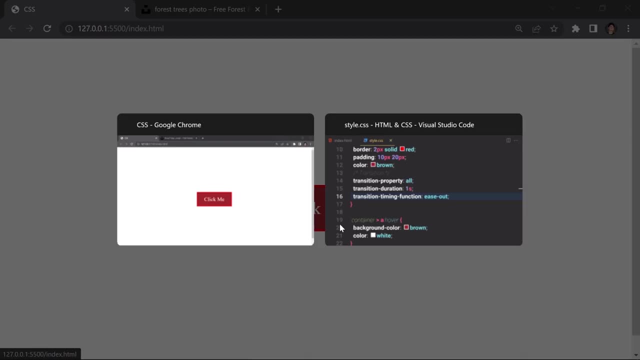 using something called ease out, maybe. and now, if you save our file, and now if i hover my mouse over to it- and here you can see this transition, if i hover my mouse over to it, so a few things happening. the background is changing and also the text color is also changing, and that's because we put 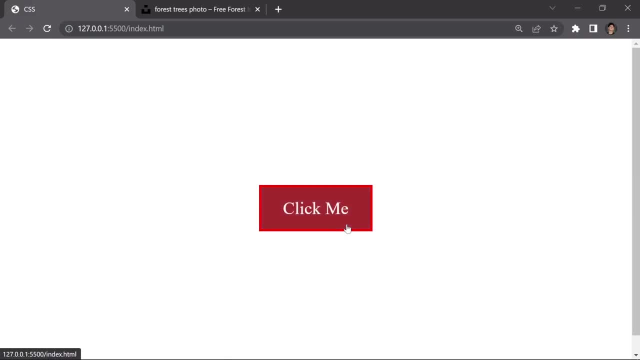 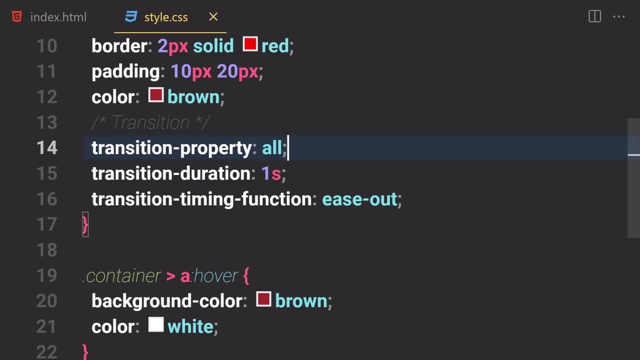 this background property of all to all of. so that's why, if you have a mouse over to it, so everything is taking a little bit of time, and everything is taking a little bit of time that's because of this transition duration property. okay, so if you set that like two second maybe. 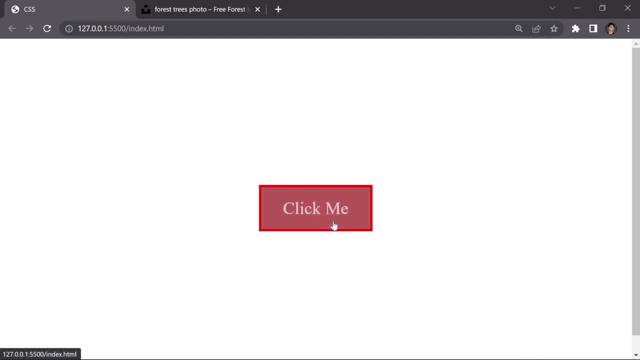 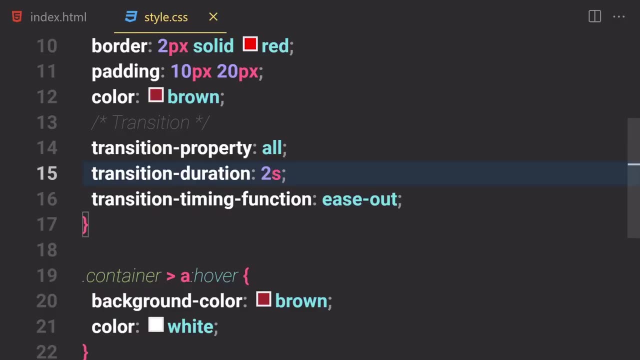 so if you save there, so now if i hover my mouse over to it, so it will now take two seconds to apply that kind of a transition to it. okay, and then we have our transition timing function and we have different kind of values for that, which we are not going to be. 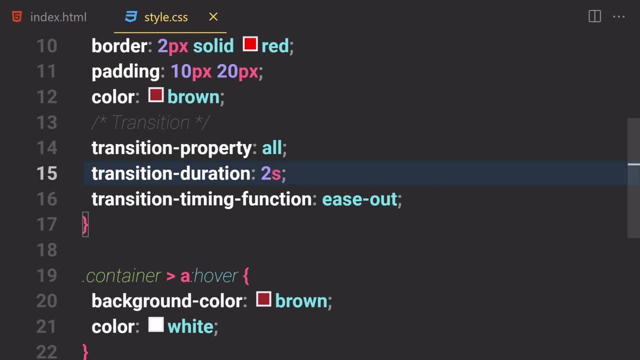 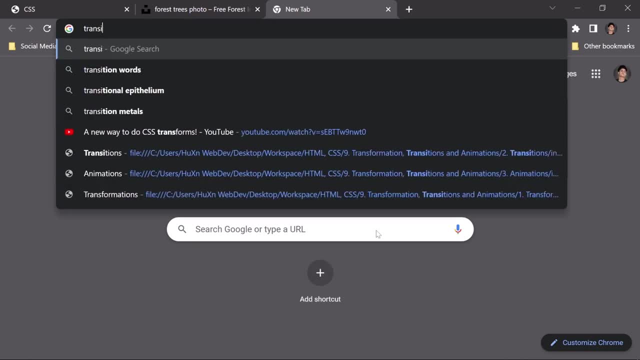 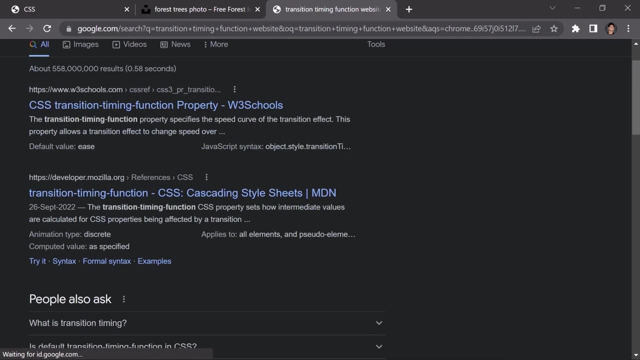 getting into because it will just waste your time and you can explore, like countless properties. and i guess somebody made a whole website about transition timing function. let me just check that real quick: our transition timing function uh website. so i'm going to just search for that. okay, so we have w3, school museum developer, and then we have the art of web transition timing. 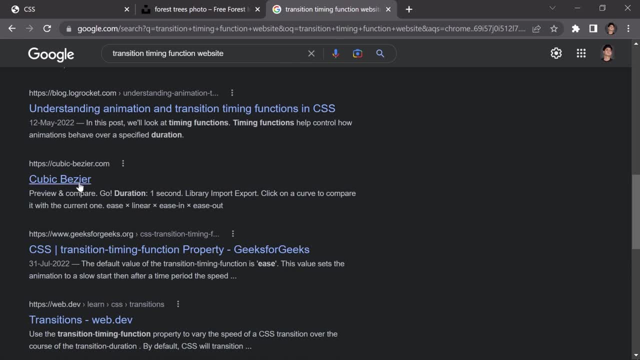 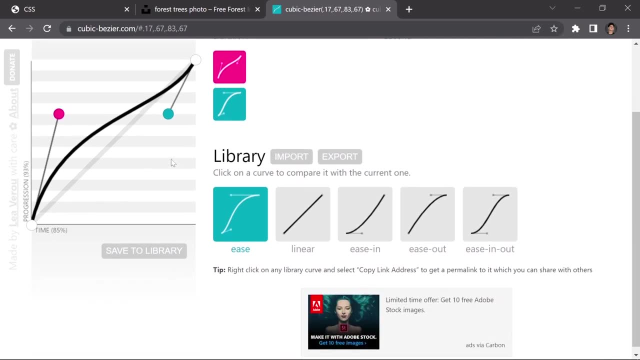 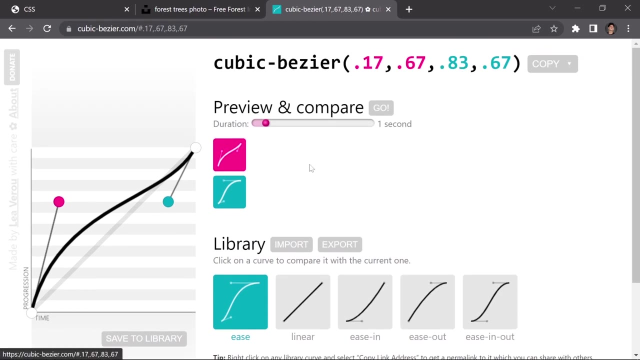 function css tricks block. okay, so, cube blazer, i guess that's the website i was looking for, all right, so here you can see we have different kind of transition right here that you can play around with there. so, um, let's just see, here is the code. you can copy that and you can put it in your css file. 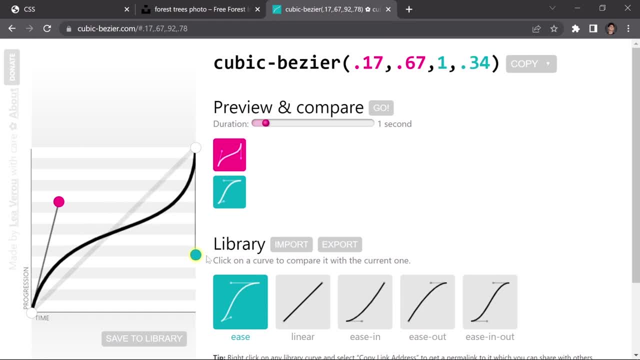 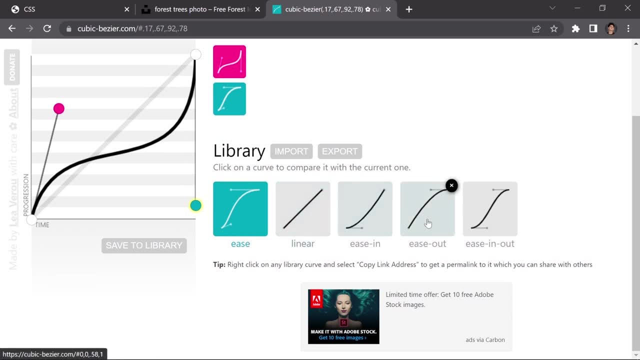 i didn't play around with this website, but i knew there is a website who allows us to put a transition. so we have different kind of transition right here. we have a ease, we have a linear is in, is out, is in and out. so now let's just use that real quick. 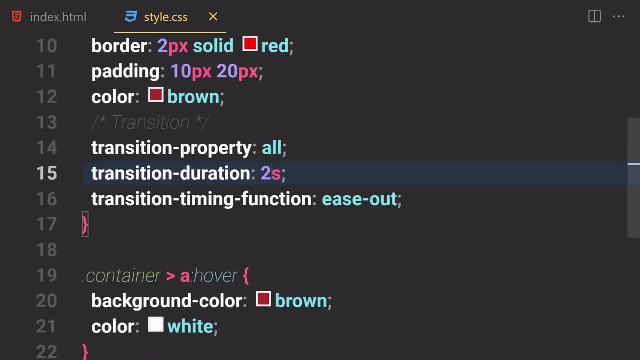 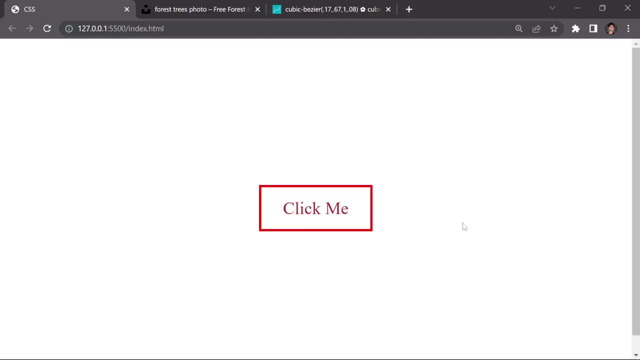 instead of using is uh, in and out like ease out. we just provide that we can just use like ease in and we set that to like one and if you save that, so that transition will apply in that fashion. so if you have a mouse ordered, so first of all, it's just a little bit slow, and so then it went through. 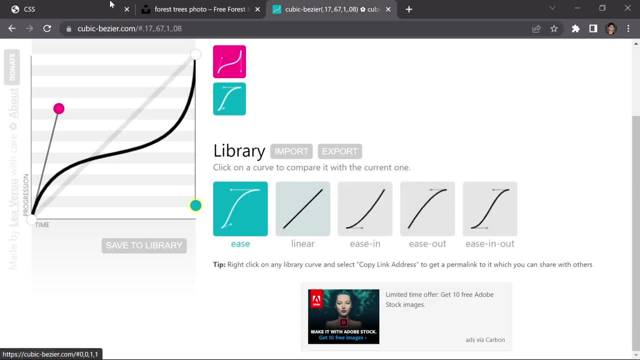 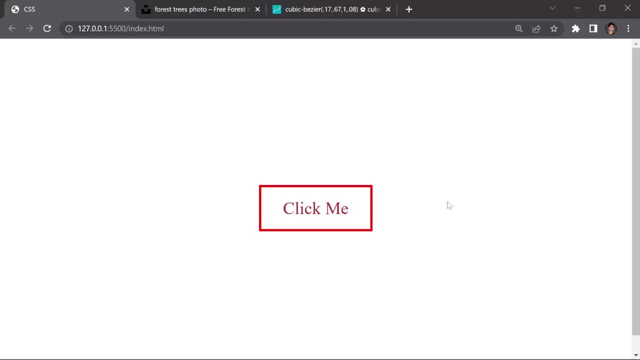 a bit fast, so now let's just copy. uh okay, so now let me just show that linear one real quickly, instead of using ease in and out, so we can just use a linear and if you sell that and if you have it will now, that transition will now apply linearly, so we can play around with this. 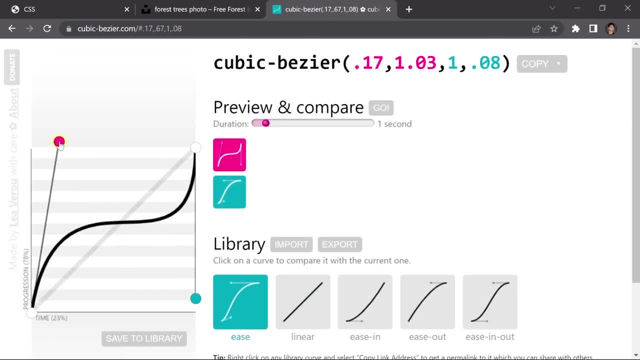 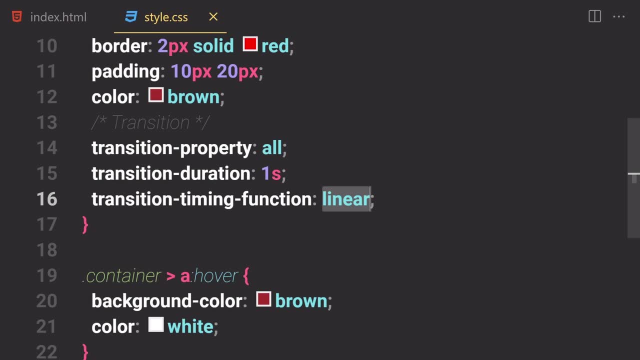 property. if you want to maybe like, if you select this kind of transition, like so, and i'm going to just click on the copy, it will now copy that code to our clipboard and if you just pass it right here, so it will now use this cubic base year. uh, function right here and it. 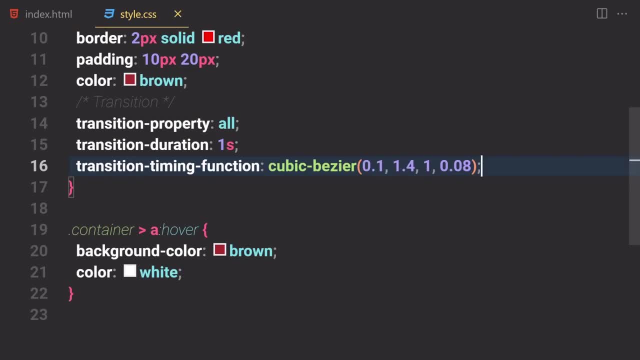 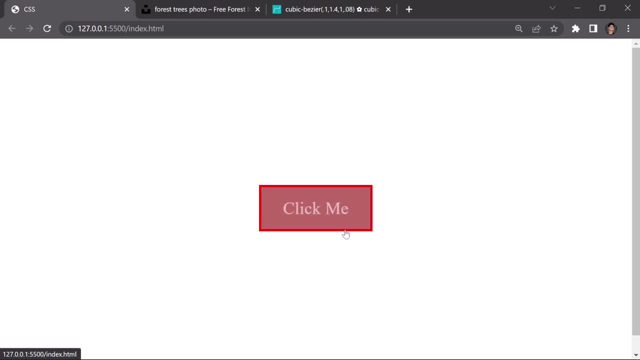 will just provide a transition timing function on that. so if you save that and now, if you have a mouse ordered, so here you can see something weird is happening. first of all, if i just have my mouse ordered, so it will take a little bit of time and then it will just push up all of the 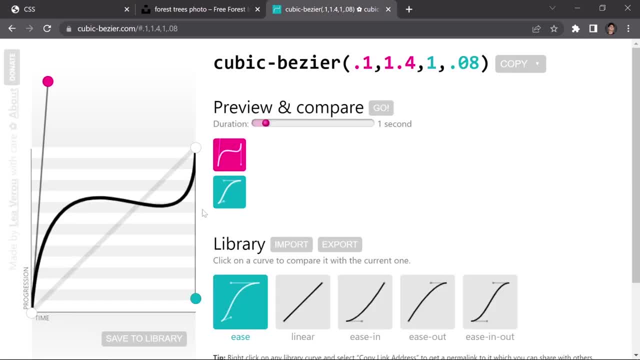 content at once right here. okay, so you can play around with that if you want to like, maybe i'm going to select everything, like so, and i'm going to make that a bit slower at the beginning and then we want that to happen a bit fast. so we can play around with that. like so, i'm going to click. 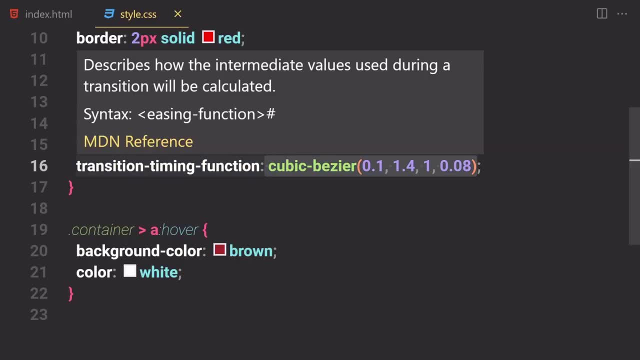 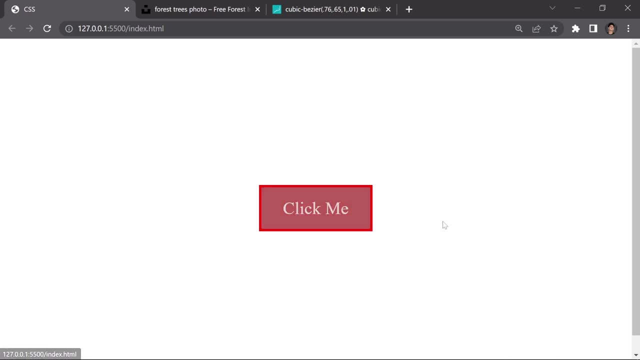 on this property or this copy button and then let's just replace it right here and if you save that, and now, if you have our mouse over to it, so it's taking a bit of time, and then it will just blink it up so you can play around with these properties. 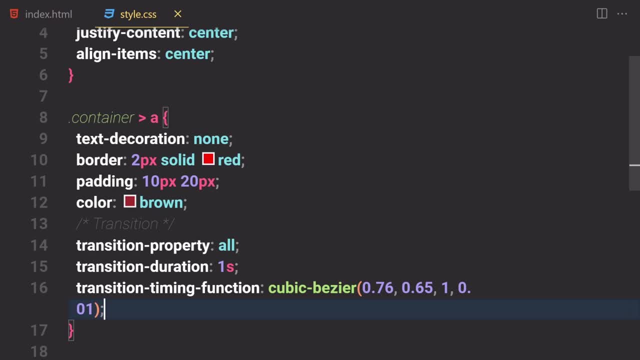 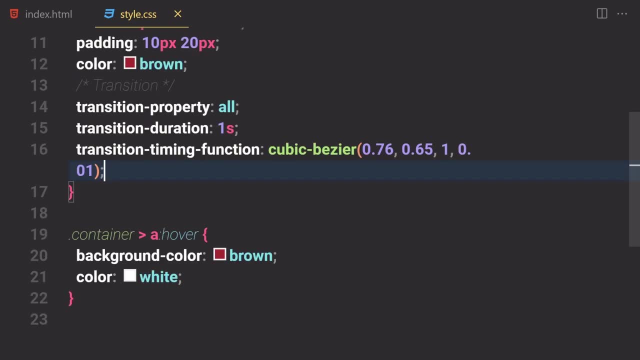 if you want to. but my job was to show you all of that stuff and now you can play around with that if you want to. so first of all, if you want to use a transition, for that, you need some sort of a changing thing. so in this case, we are going to be changing or things by using a hover. uh, 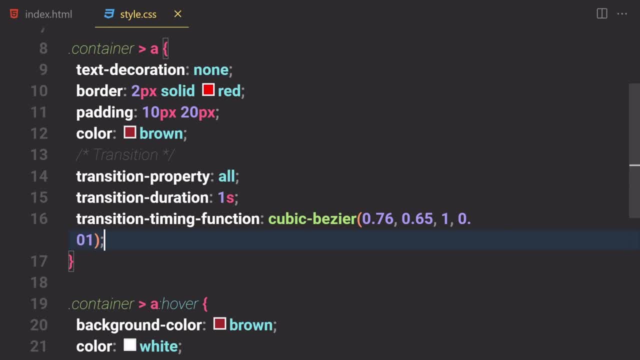 pseudo selector. so then we can use a transition properties so we can just change the transition of one thing or we can change everything by using an all value. then we can also specify a duration for our transition, like this will be the time of our transition, and we can also specify a different kind of function for our transition. so now we are. 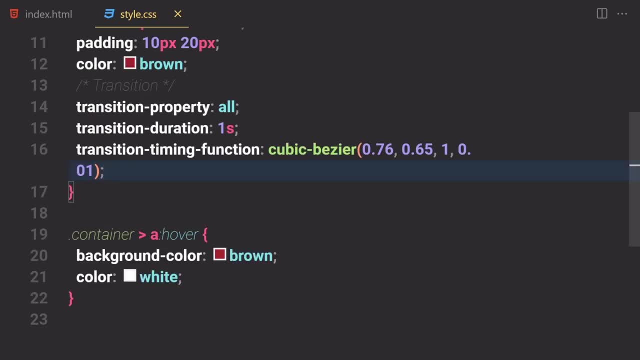 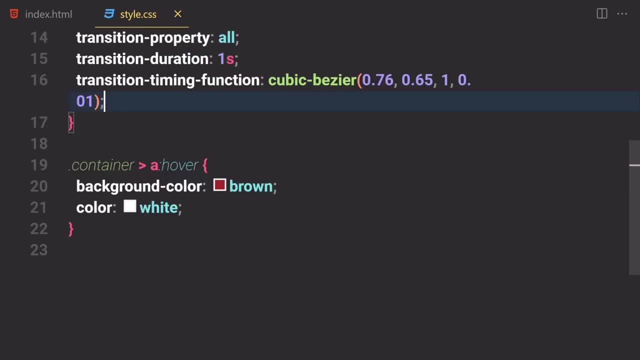 totally done with the transition side of this video. now let's just learn about, finally, something called animation in css, and we are not going to be building awesome animation, but i just kind of want to show, is that how you can create animation, just a basic syntax of animation. so now, if you 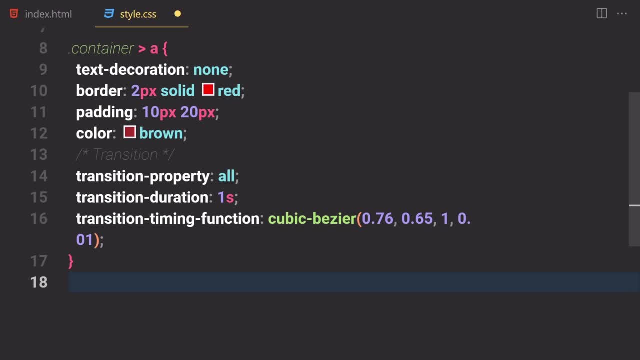 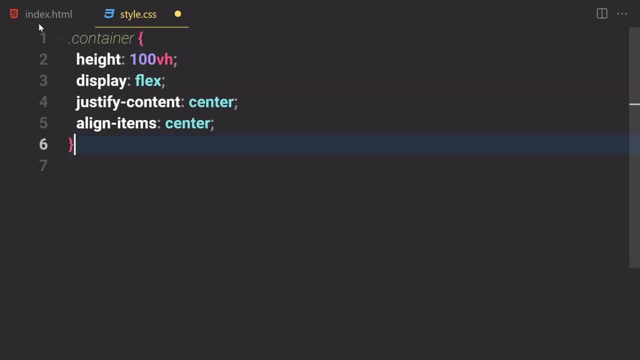 want to learn about animation. so i'm going to remove this column from here and i'm going to also remove all of these transition stuff from there. and you know what? i'm going to also remove this container and anchor tag and also remove that anchor tag from there and i'm going to replace it with div. and now we are. 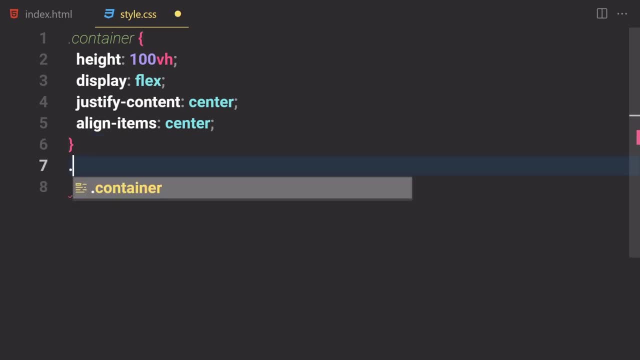 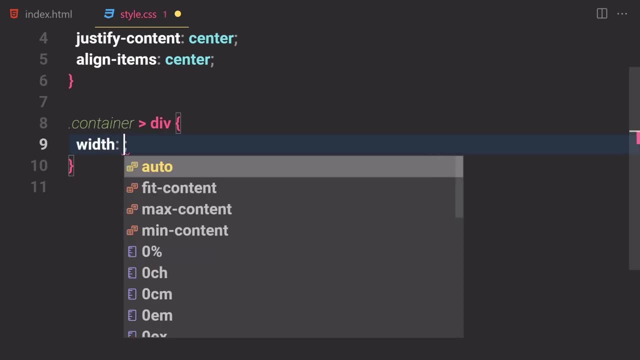 totally good to go for now. all right, so now let's just select our container real quick and then everything inside that container, like all of the div which are currently available inside that container. let's just give them a width of like uh, let's just provide like 300 pixel of the. 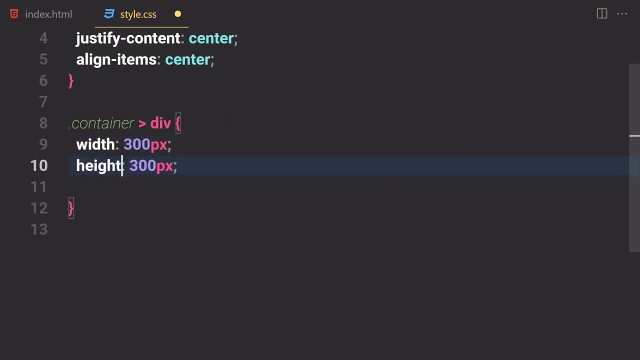 width and let's just duplicate that to the height as well, and i'm going to give them a background color of like dark blue color. and now in here we are going to be starting over and knee motion. so before we start animation now, let's just learn that. what in the world is animation? 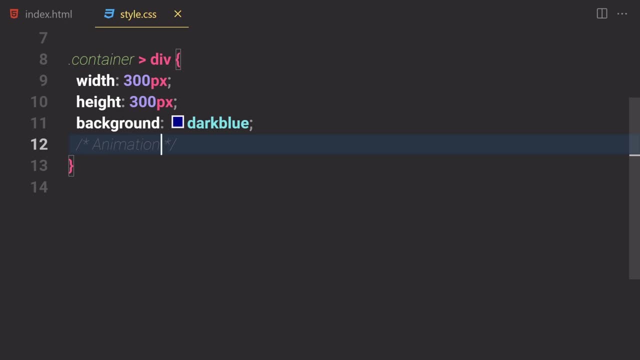 so animation lets an element gradually change from one style to another. this is what animation is. you can change as many css properties you want, as many time you want, in a keyframe. so what are keyframes? so, anytime you want to create your animation, so for that you need to work on a keyframe. so we are going to be using our animation stuff. 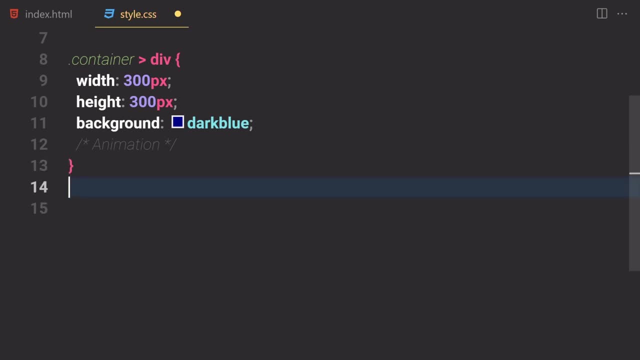 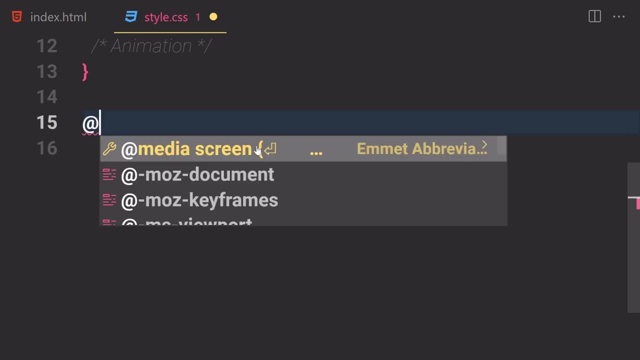 or animation property in here. but first of all we have to create our keyframes. for that i'm going to zoom in a bit. and now, if you want to create an animation, first of all you're going to be writing add symbol and then key frame. okay, so if you just write a keyframes in there, 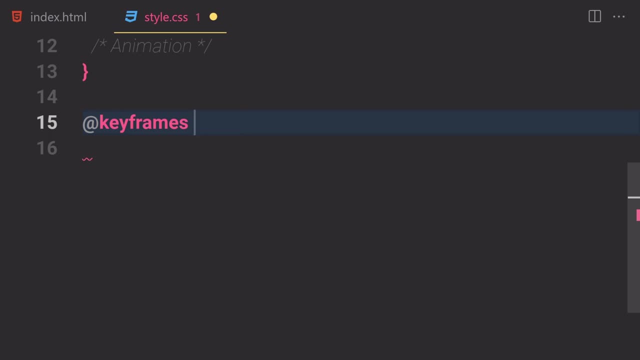 then provide a name for your animation. so in this case, i'm going to just give a name of like uh, i don't know, i don't have any animation in mind, so i'm going to just give like a random word, like in and out, and you can give any name you like. you can give him hosan. 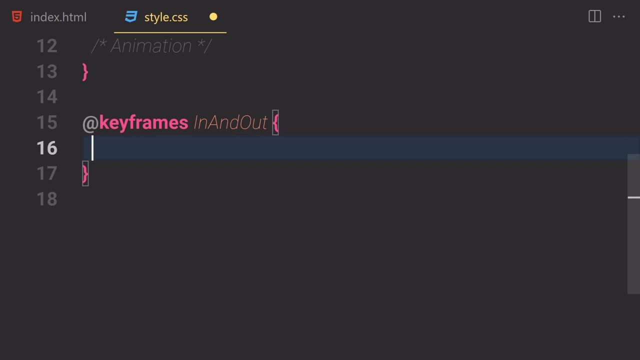 animation if you want to. hosen is my name, by the way, and so here we can specify that from where or animation should start, so we can just write like a zero percent, or we can also use like a to and from keyword. okay, so you can also learn about that if you want to, but we are going to be just using. 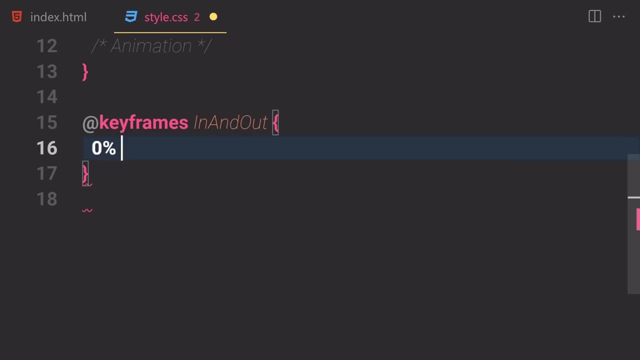 like zero percent. so animation start from zero percent and you know what? what should we do in this zero percent? i'm going to just use like maybe transform or scale something. i'm not sure what i'm building right now, but i'm just showing you what animation is and how to work with that. if my animation was horrible or 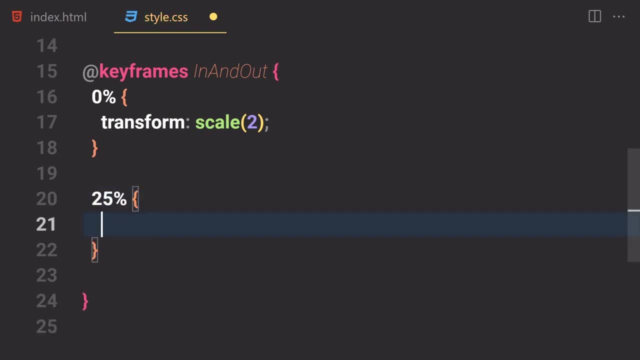 an awful. you can create your own animation- awesome, but mine will be awful. so we can work with like zero percent, twenty five percent, ten percent, twenty percent, thousand percent, however you like, but in my case i'm going to just go from zero to 25 to 50, okay, and i can also go like other. 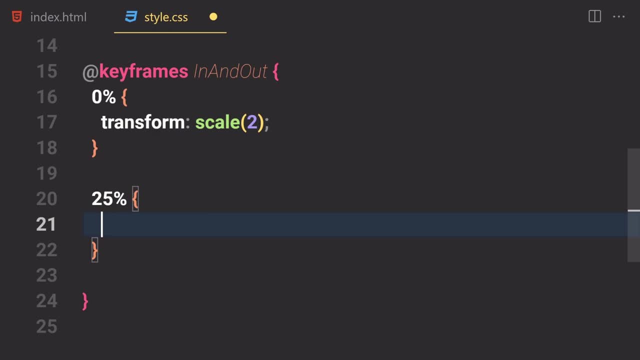 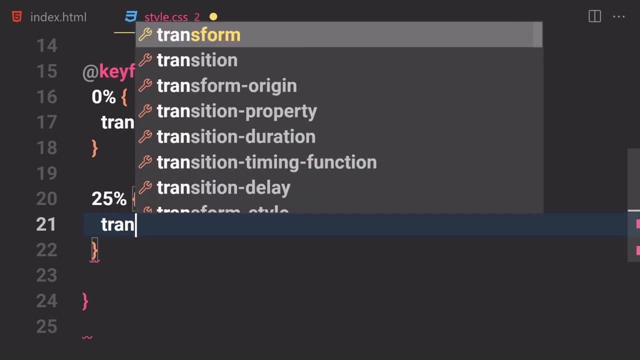 direction if i want to, so this one will be. this one is the first frame right here and this one is now the second frame, and you can create as many frame as you want. so i'm going to just use like transform in this case and i'm going to just provide a scale of 0.2 and then background color. 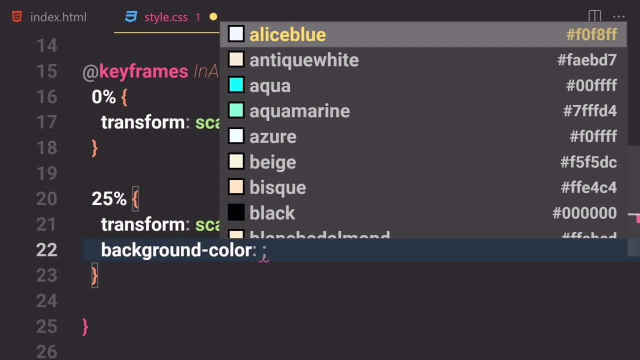 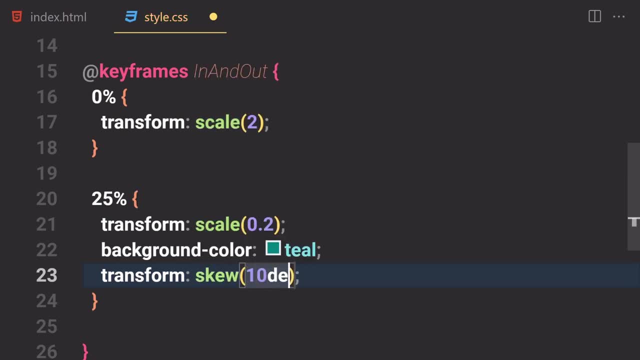 i'm going to change the background color to be like- i don't know. i'm going to write like teal, maybe in this case. and now let's go to the next one. just use a transform of skew and we'll just keep up. or animation, i know this animation will be. 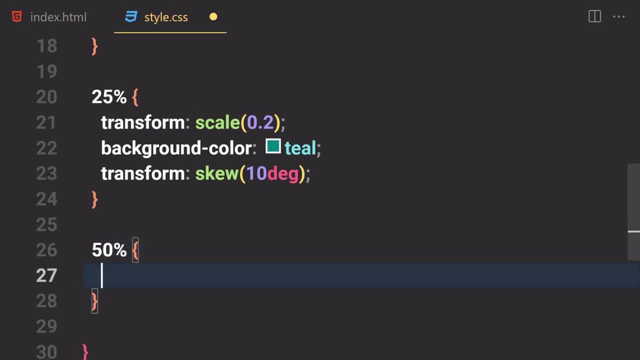 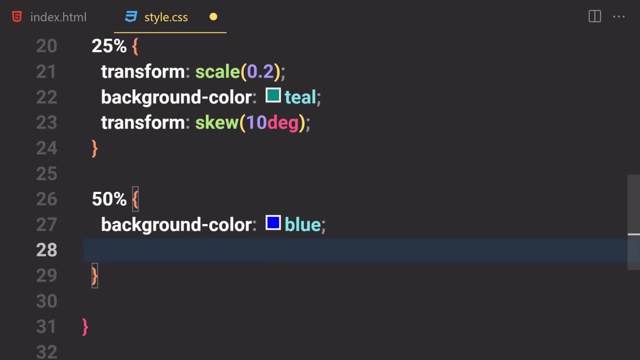 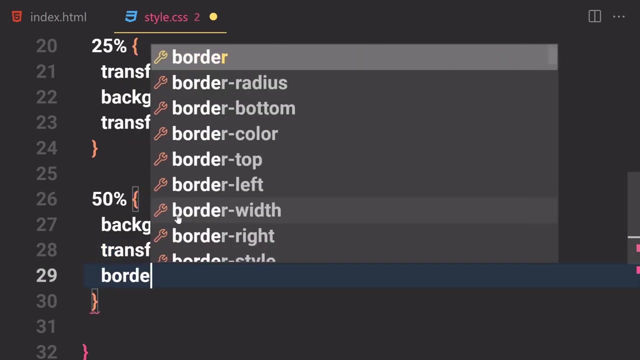 totally awful. and now let's just use 50 in there. and now let's just use background color to be like, uh, i don't know, uh, totally blue in this case, like in this frame. and now let's just use our transform and skew it up one more time to the 40 degrees and border uh radius will be 50. so if you 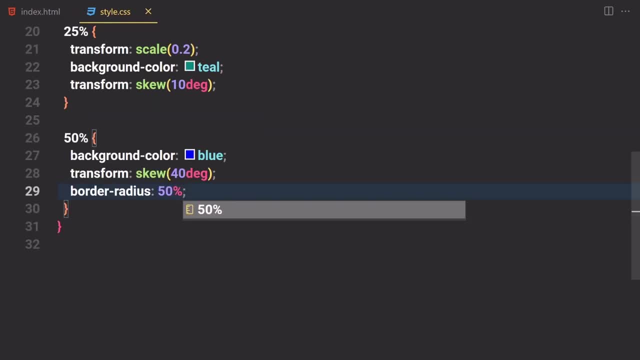 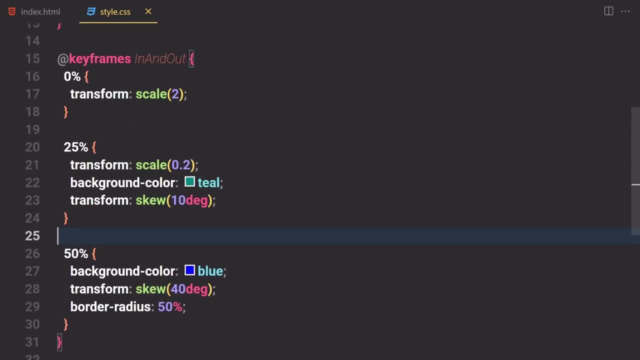 just use that now if you save our file. and here let me just say that now we totally create our animation right here. so this is how we can create our animation. so how can we use this animation? so now, if you want to use our animation, so first of, 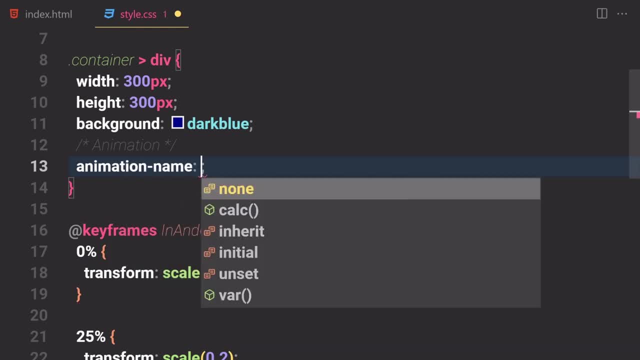 all we have to provide the animation animation name. so what is the name of your animation? in this case, my animation name is this: in and out. so i'm going to just copy that and i'm going to paste it right here. what else do you have to do? how much time or animation would take? so we are. 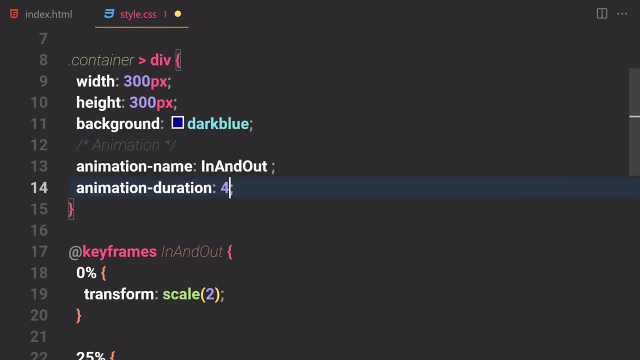 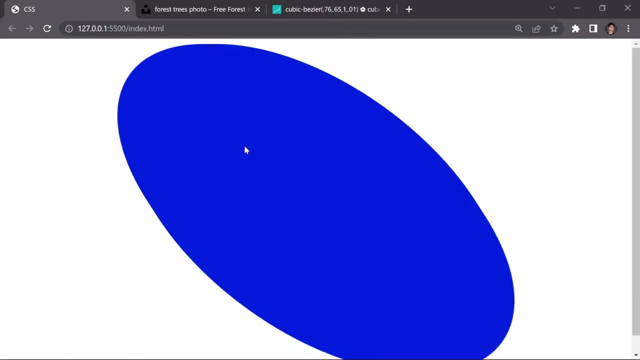 going to be just specifying like animation, animation, animation, animation, animation, animation, animation. duration of four second would be fine, so i guess that would be fine. so i'm going to just save that for now, and here you can see my animation. it's horrible, i know. uh, you can like create crazy. 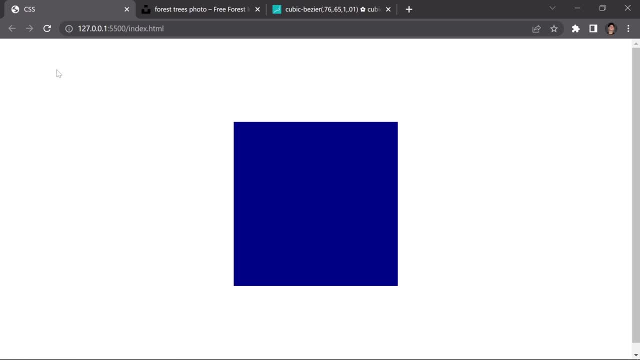 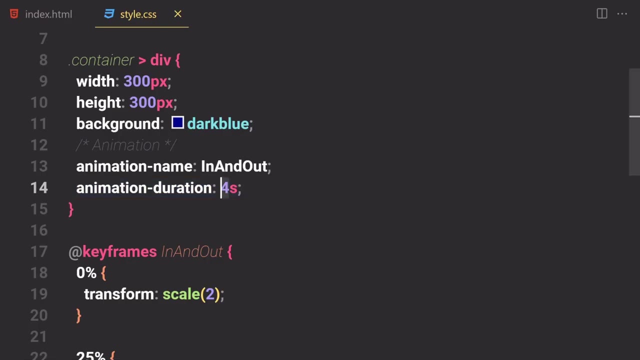 kind of animation if you want to, but in my case, uh, i just create this awful one, so i'm going to just refresh my browser and, by default, everything looks like that, if you just refresh it one more time. so this is how we can play around with our animation. so, instead of providing like four, 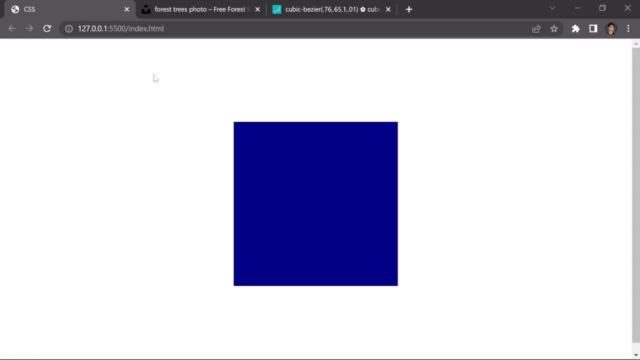 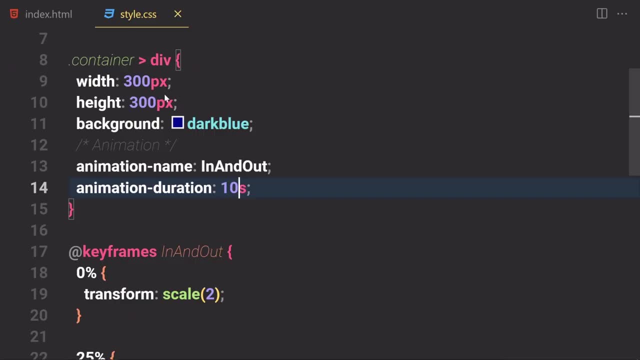 second of duration. we can also make it faster by just writing like two second and if you just refresh that and our animation will happen in two second. we can also write like maybe 10 seconds. so if you save that and now our animation will just happen slightly slow, you can just play around with. 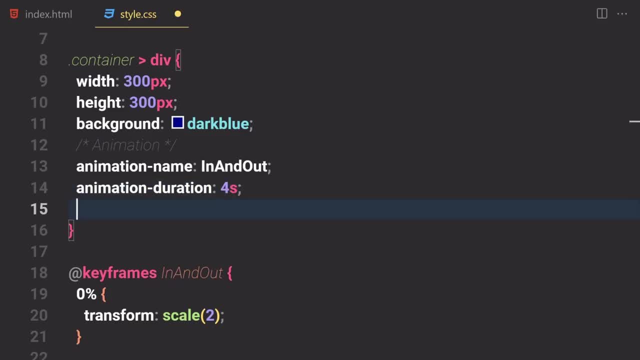 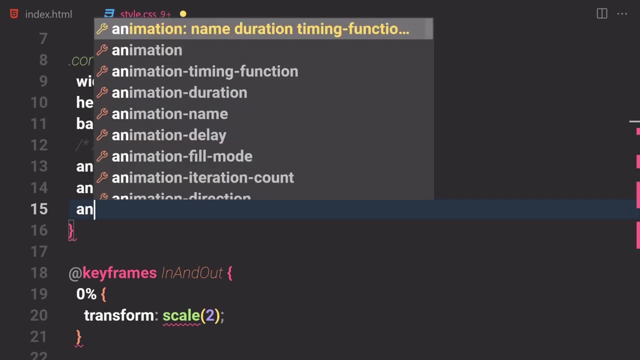 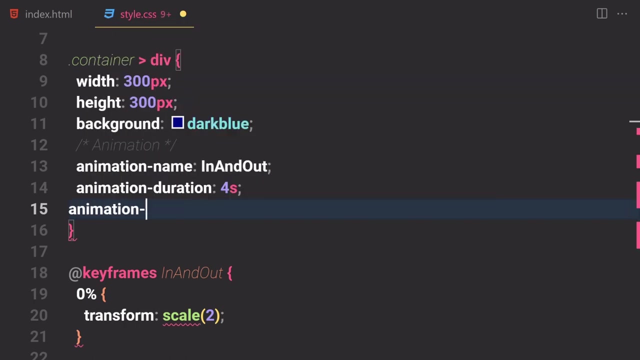 these properties if you want to. so now, the next property which you are going to be learning about in this section is something called animation iteration count, and it allows us to run or animation the amount of time you want. so you're going to be just using, like animation, uh, animation, iteration. oh my goodness, animation, iteration and count. 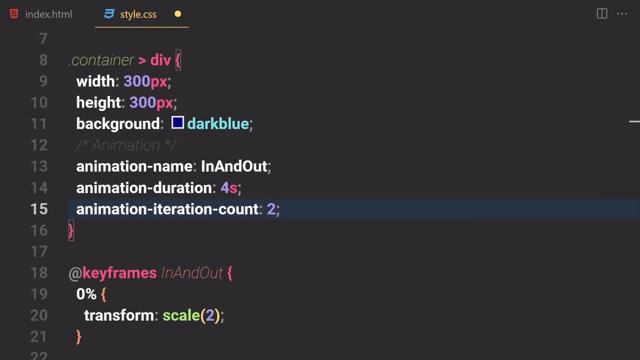 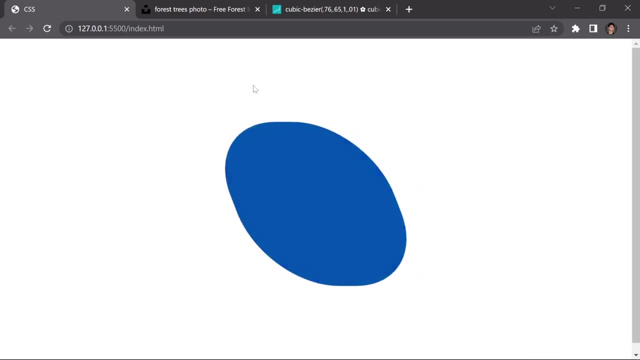 all right. so this is what i meant and here let's suppose, if you just specify like two times and if you save that, so it will just run or animation the first time. so let's just save that and refresh. so this is the first time of running our animation and this is the second time and it will just stop. 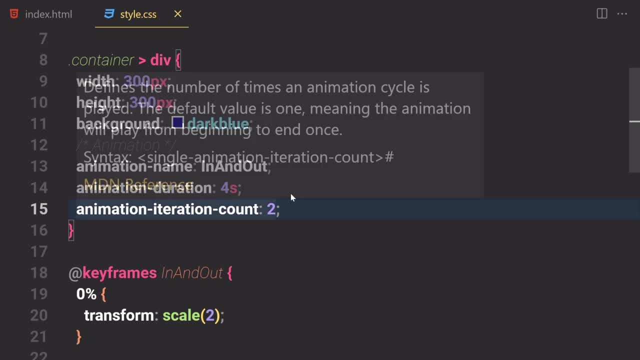 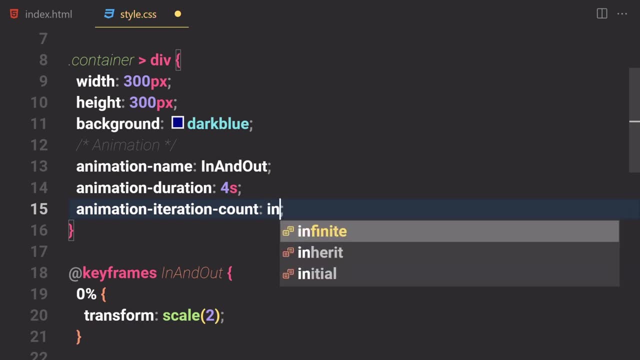 okay, so we can specify how many time we want, like we can provide five thousand, how many we want. so if you want to run this animation like infinitely, so for that we can just use like infinite for it here. so if you just specify infinite and save it, so this animation will. 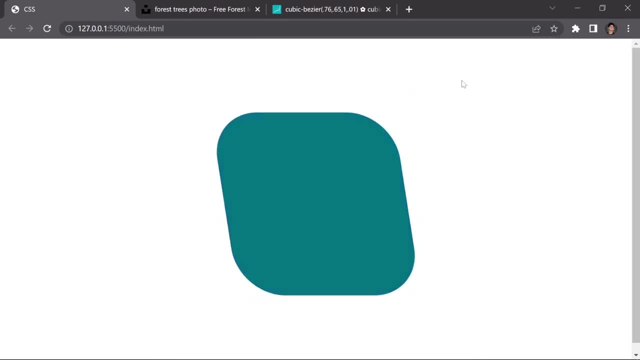 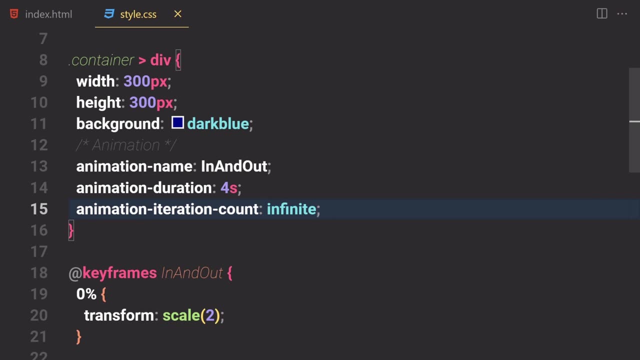 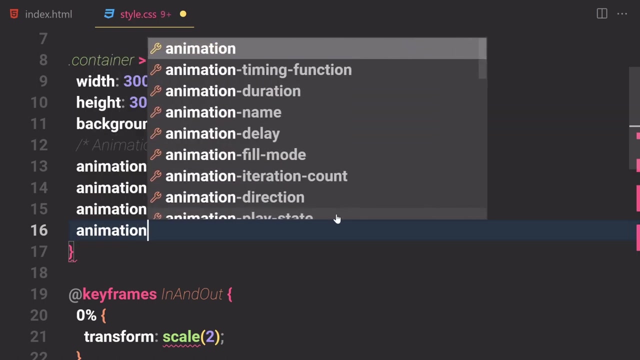 just run again, again, again and again, like infinite time. okay, so this animation will run like infinite time. you, and this is how we use animation- iteration count. all right, so now the final property which we are going to be learning about is something called animation. animation, uh, timing function, oh my. 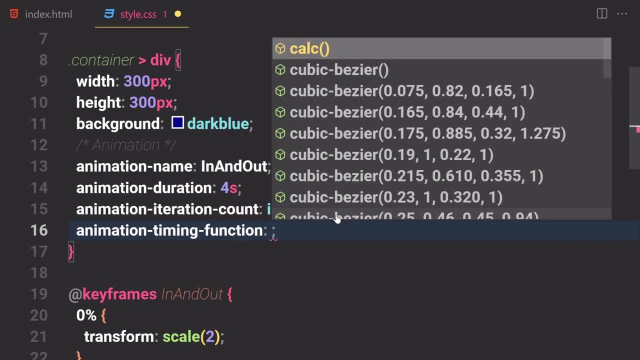 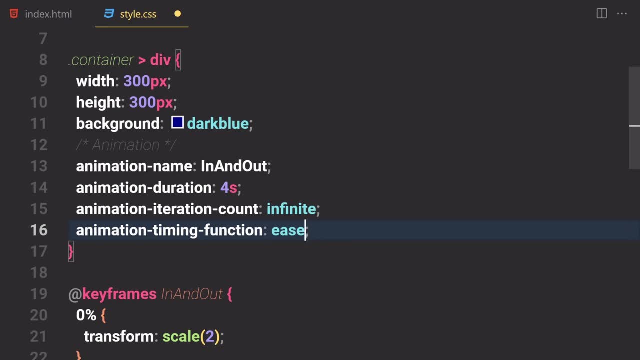 goodness, let me just write this timing function real quickly and here we can just use that: is in, is out, is, uh, whatever is in and out. we can also use that linear if you want to, but in this case we are going to be just working on is in and if we save that, so our animation will happen slowly. 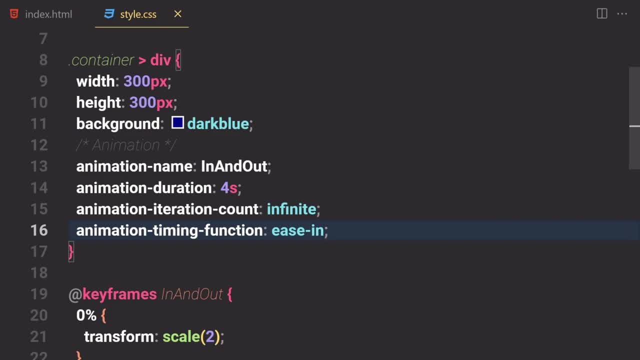 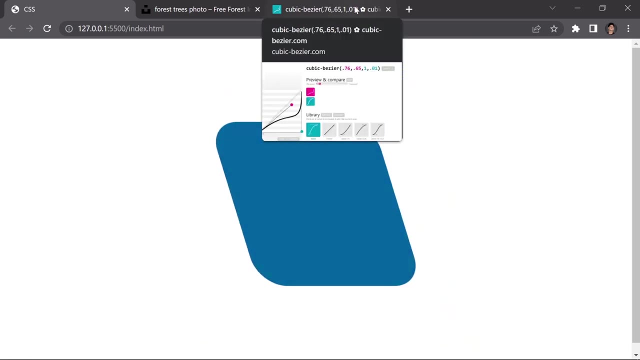 and it will just um go fast like so, and then we can also just play around with this cubic base. yeah, if you want to, and now let me just paste that in here- and if you save that and boom, boom, so our animation will happen like strangely, we can work with that cubic base here a little bit more, if you. 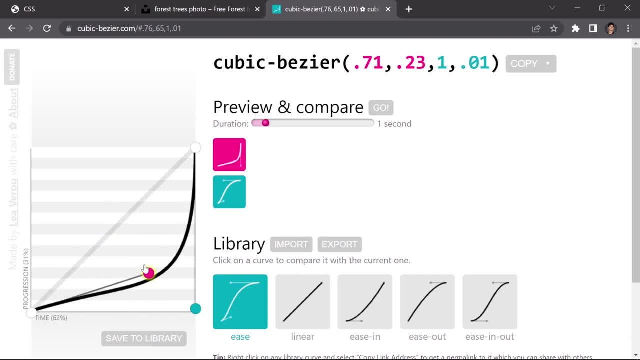 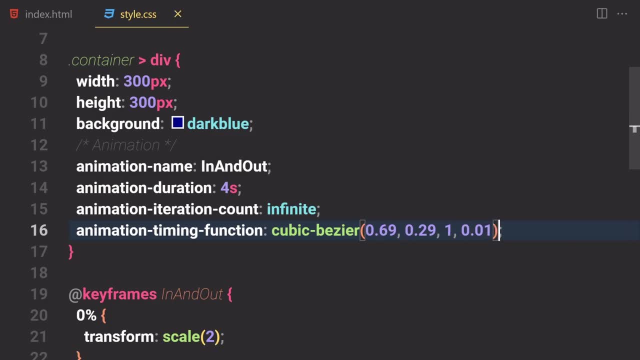 want to, and i will never recommend you to spend a lot of your time because you're not going to be spending a lot of your time on cubic base- yeah, in a real world project. so i'm going to just paste that there right here, and, if you save that, and this is how it will look like first of all start. 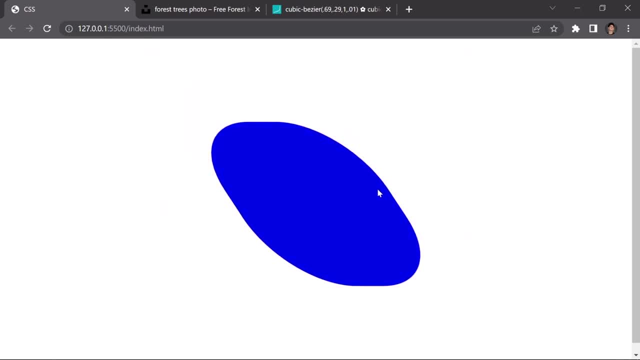 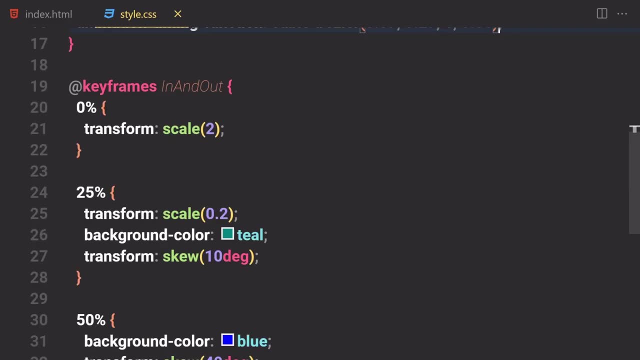 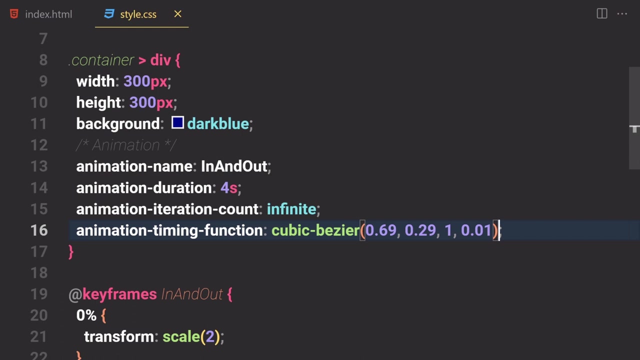 very quickly and then slow it down, like so, or slow down very quickly and fast. i. i don't know what's happening in this animation and, by the way, it's a awful animation which i created. you can create awesome animation for your project, but now we are totally done with animation and everything. 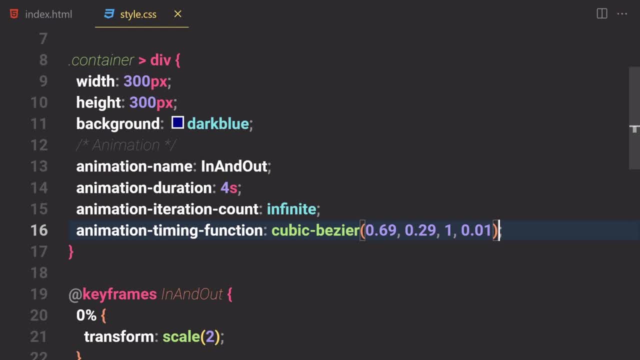 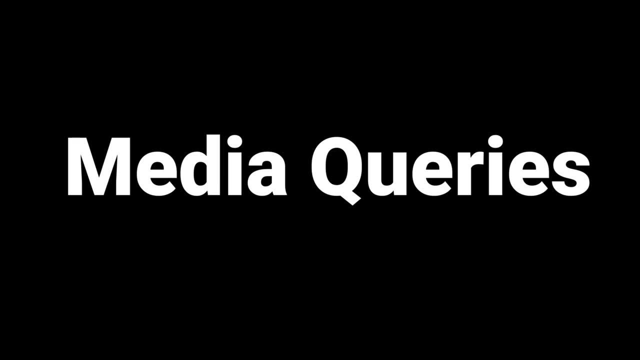 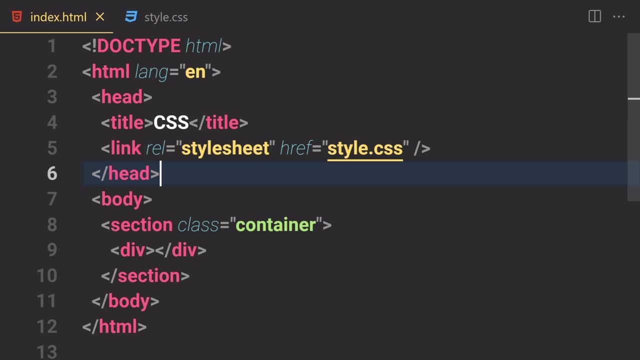 so i guess the final topic in this course is left, which is called media queries and which you are going to be talking about next. all right guys. so if you're already here, then congratulations. you're not at the end of the schools. so now there is just one topic left, which is called a media queries. 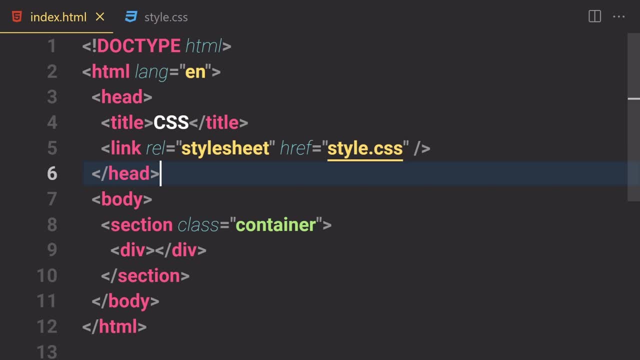 which you are going to be learning in this section. so now, what in the world is a media query? so media query allows us to provide different kind of styling for different devices depend on their features. so what do i mean by all of that gibberish which i just said? you know what i'm going to just 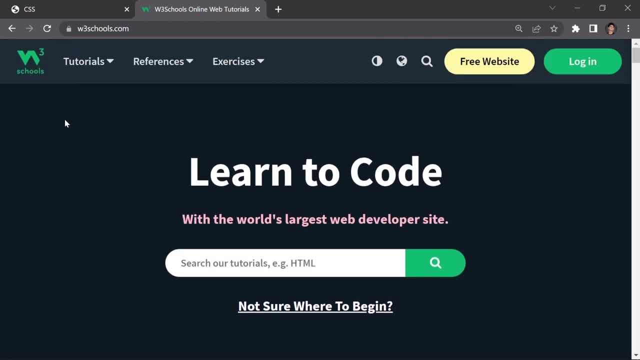 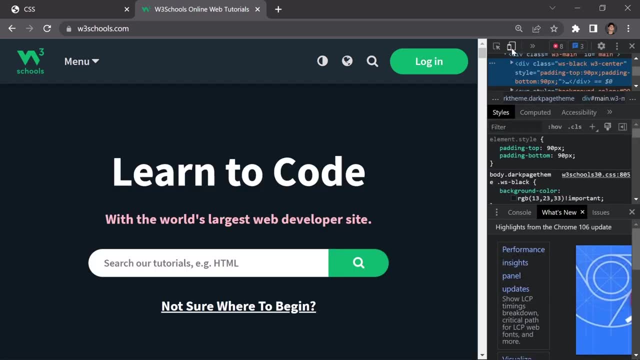 go to the w3 landing page right here, and then i want you to just right click on somewhere and then click on this inspect area. so if you do that, here you would found this uh tablet and this iphone kind of a toggler. so if you just click on that, so it will now allow you to check this site on a different 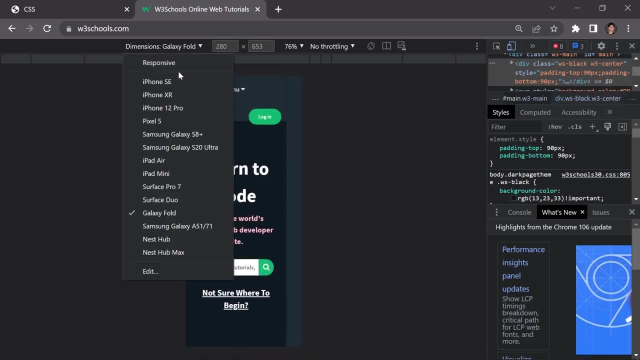 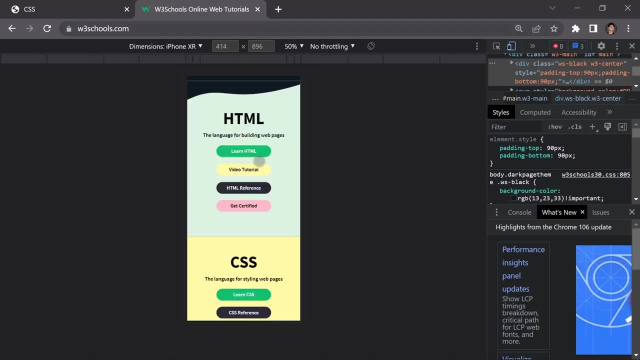 kind of screen sizes right here. okay, so we can just check it for i don't know, like for iphone se, and this is how it will look like on this iphone. this is how it will look like on an iphone xr and a lot of different kind of devices we have right here. 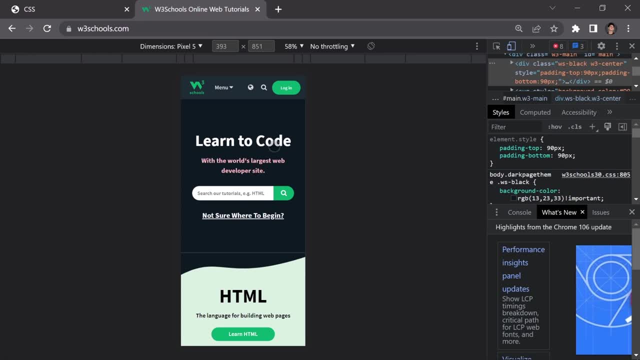 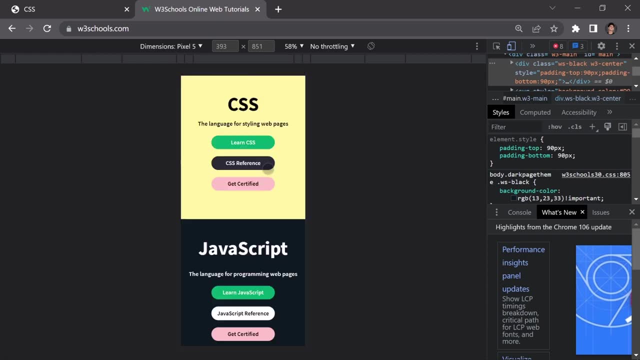 we can check it for a lot of different kind of devices and this w3 side is totally responsive. so that's why we are seeing like everything in just one page right here. so if this site was not responsive, then you would just see like a clunky, weird thing. okay, and by the way you know, 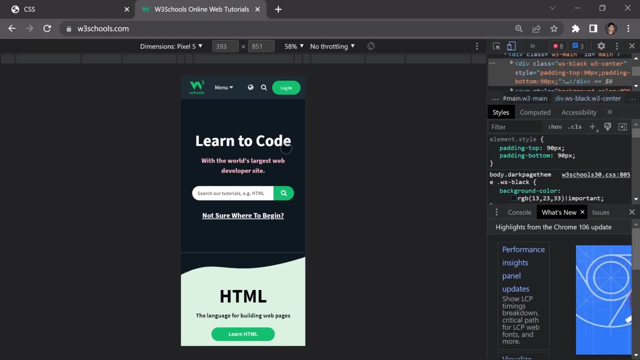 if on any website online which is like not responsive nowadays, nowadays if you want to push your site into google and stuff, so you have to make it responsive so that it will work on a different kind of uh screen sizes like more or more than that you can easily check for a lot of. 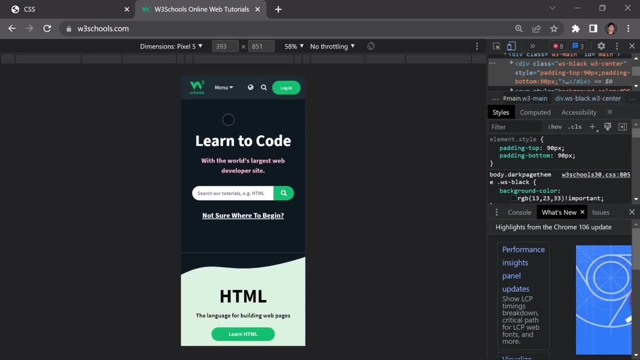 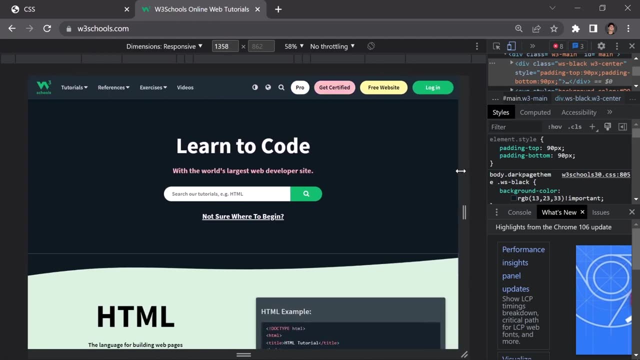 mobile, tablet, uh, iphone and a lot of different kind of devices. so you can just click on that and click on this responsiveness right here and here. it will allow you to just check it on a different kind of screen size right here here you can see we have different kind of uh. 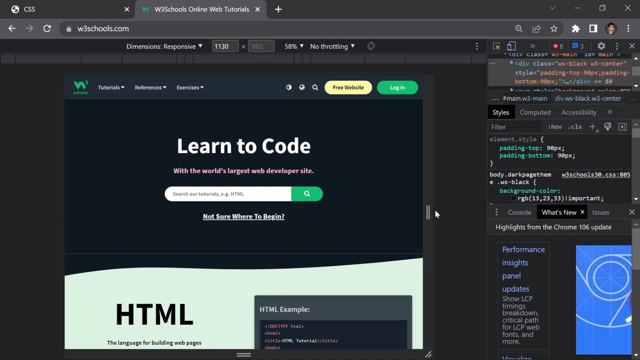 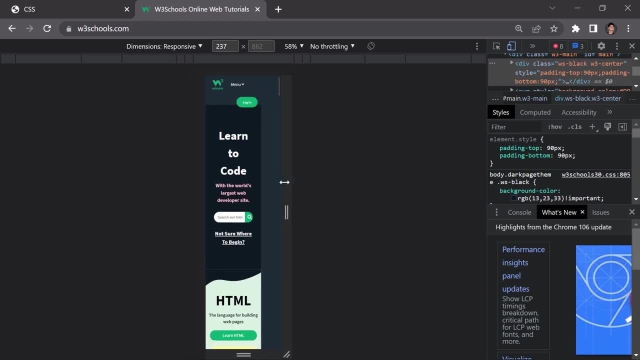 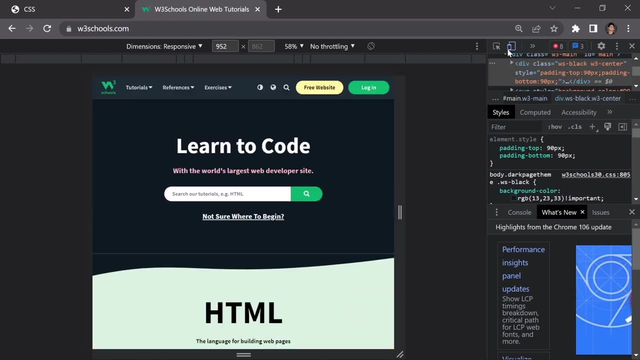 icons like a tutorial, references and exercise. if you make that smaller, so that will be gone. so we have menu right here and so on and so forth. so this you can check it out, different kind of websites and different kind of things by using just these developer tools. so this is what we. 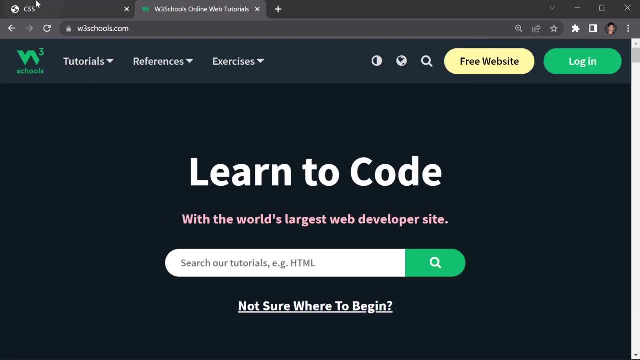 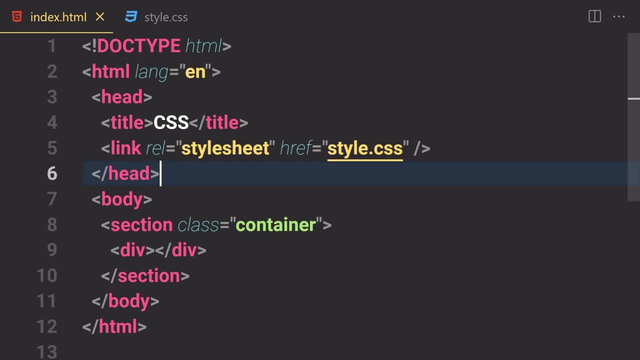 are going to be learning. we are going to be making our sites totally responsive. you can either make your website responsive by using a media queries, and you can make your site responsive by using advanced units like m, rem and percentages, signs and stuff like that. so what do i have to do? i'm 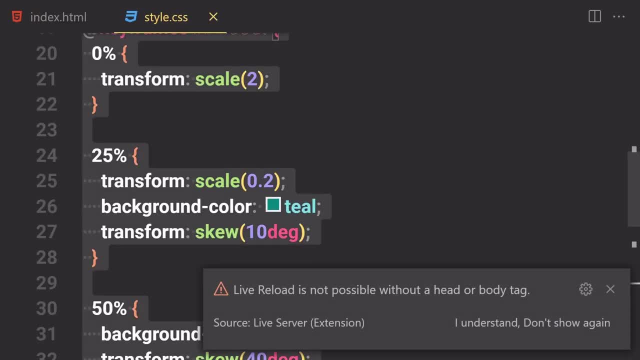 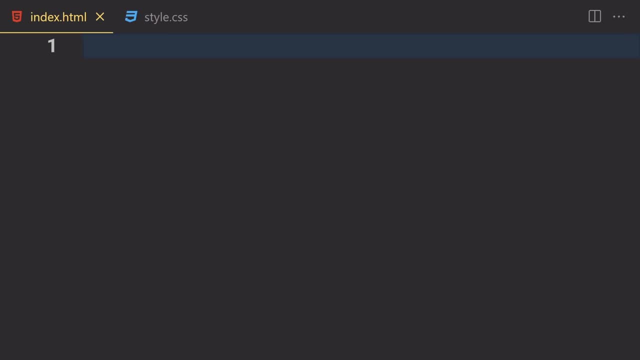 going to remove everything which i have inside my html file, and i'm going to remove everything which i have inside my css file, and i'm going to remove everything which i have inside my css file for this tutorial. all right, so what i'm going to do is that i'm going to just hold shift and then i 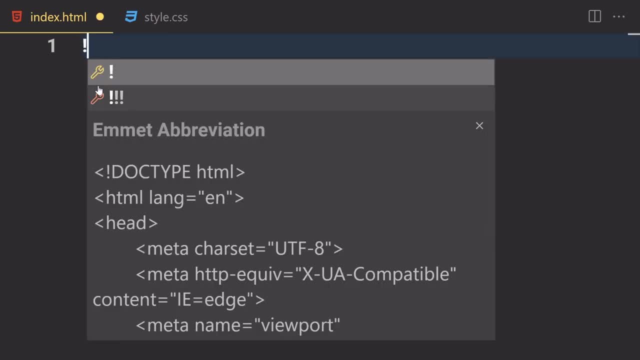 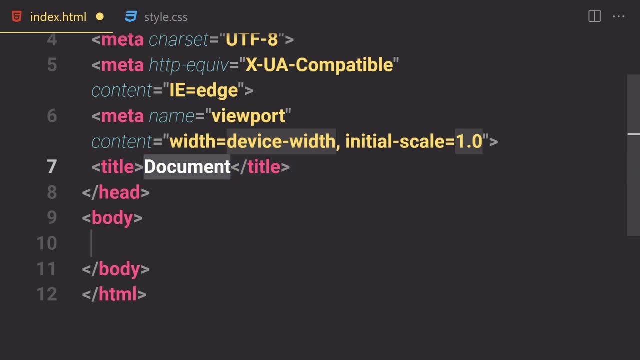 want to just hit. one certain log uses this explanation mark and now, if you click on that, so here you can see it, along with this metadata and all of the structure of html. so i'm going to just change the name to like css right here, and you should do the same so that it will use that. 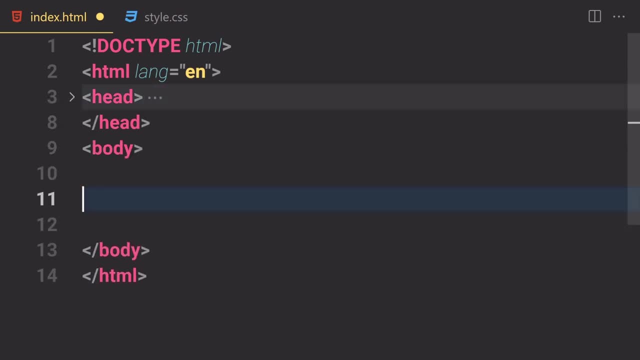 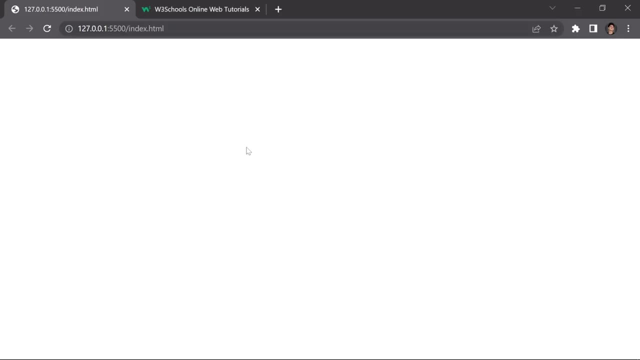 metadata right here. so if you just make that a bit smaller, and now what do we have to do? so for this section i'm going to just write h1 of media queries. so now, if you save that, so here you can see: all right, so something went wrong. okay, so it's working. let's just remove. 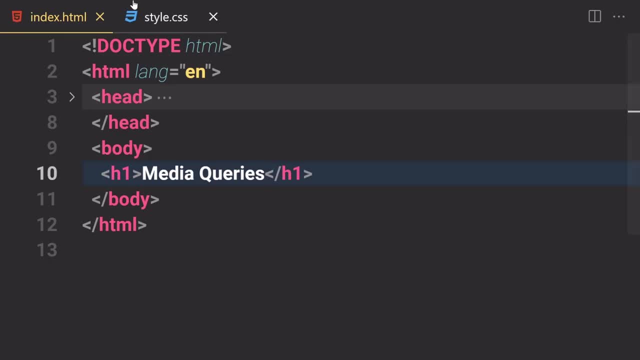 this media query. okay, so it's working, all right. so now let's jump into our css style sheet right here and now. let's just start working on a media query. so first of all, i'm going to just write a body of background color and it will be now totally set to like coral maybe, and i'm going 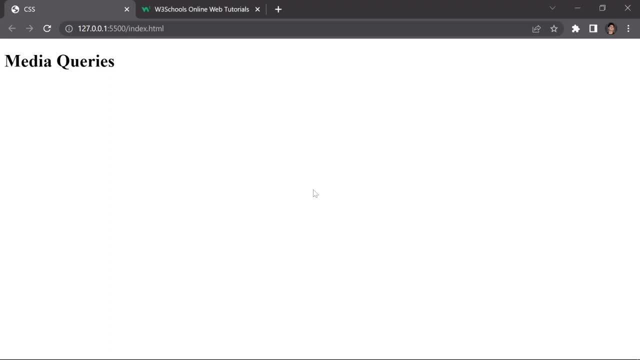 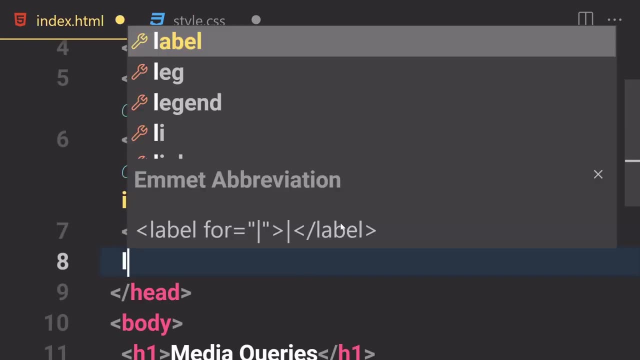 to also. you know i'm not going to change any font style and stuff, so this is how currently things looks like. okay, we should also have to link or css file file as well, and now let's just provide that link and now we're totally linked and if it's, our file. 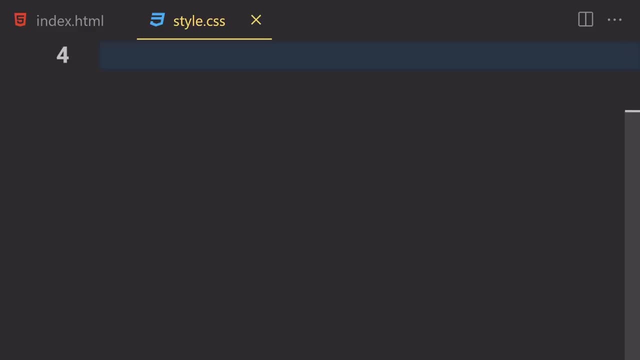 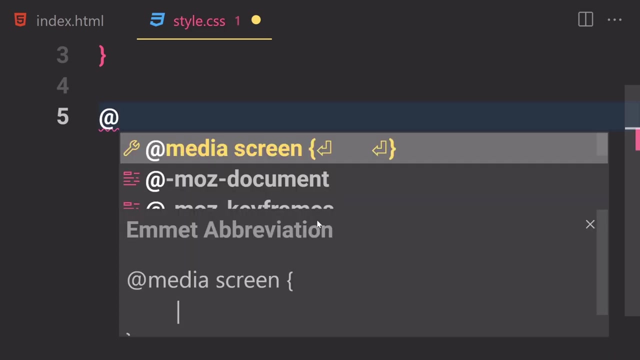 and this is how currently things looks like. now, if you want to provide a different kind of media queries for a different kind of screen sizes, so for that first of all, you just have to write an add symbol and it will give you a lot, a lot of properties right here. you don't have to worry. 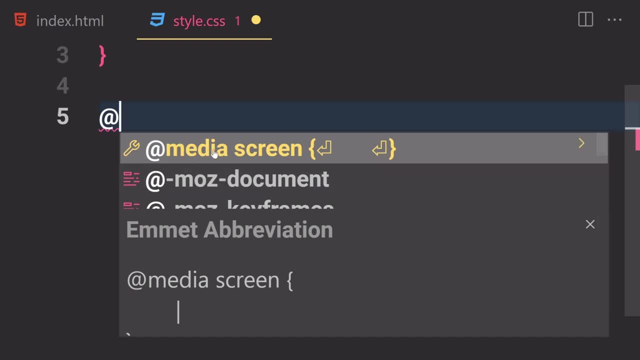 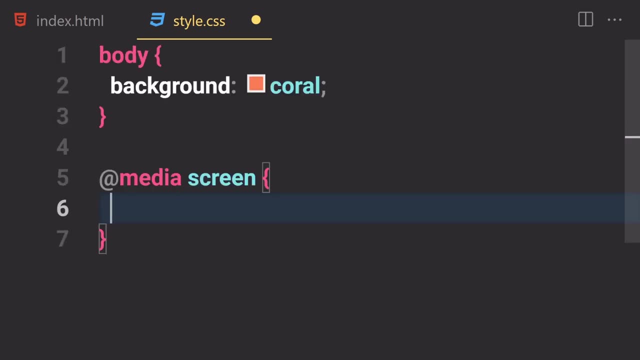 about any of them. for now, you just have to either click on that or you can write it manually if you want to, but in my case, i'm going to just click on this media and screen right here. so what is that even mean? like a media screen? so this means that we are going to be writing a lot of word styling. 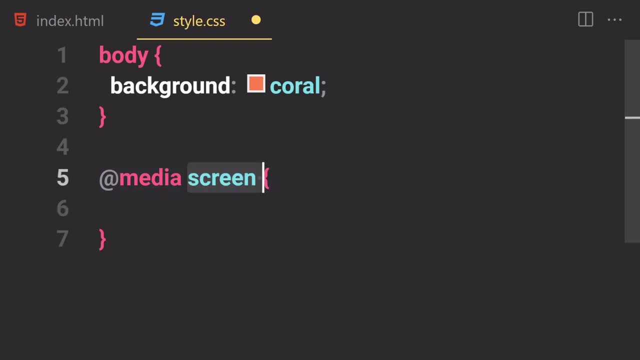 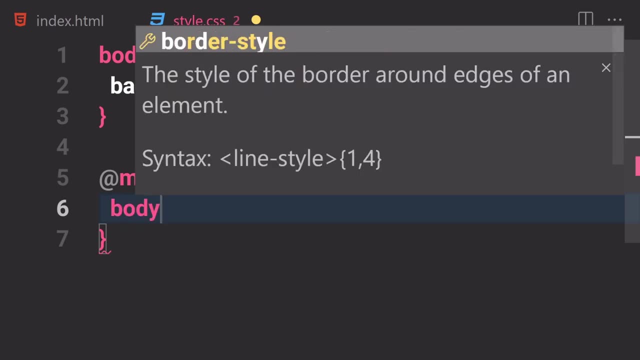 inside there, and this styling will be only for the screen size. we can also write a different kind of styling for a print, which i'm going to show you just in a second. so you know what? let's just start working by selecting our body right here. so if you now select our body, let's just write a bg like a: 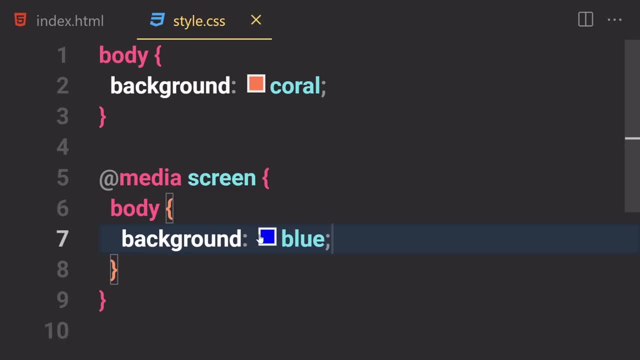 background color. and now let's just change the color to be like blue. and now, if you save that, so what's happening right here? we now just change this coral color to this blue color right here. so why is that? that's because we use this media of screen right here and we can specify. 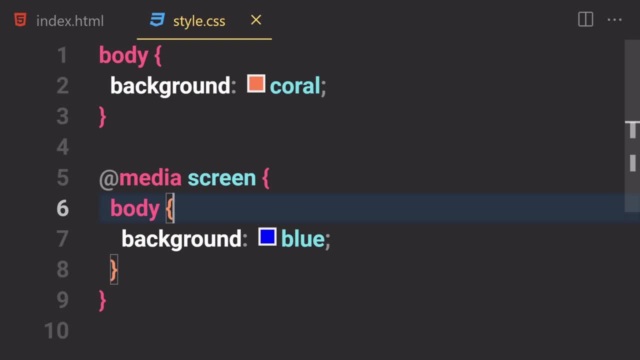 a different kind of medias, for a different kind of viewports or a different kind of screen sizes, if you want to. so to do that, first of all we just have to write, and in here, so we just write, and then write an opening parenthesis and closing parenthesis. and now, inside these parenthesis, 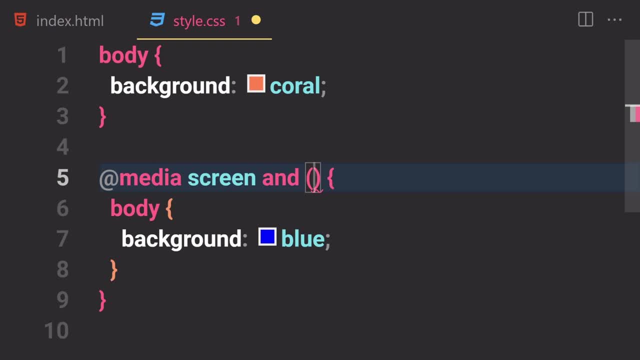 then specify the viewport width right here, so we just write, and then write an opening parenthesis right here. so let's just try like: uh, i don't know, i'm gonna just write like max width of uh, 1000 pixel right here. so if you just write 1000 pixel, so what is all of their media query even mean? so? 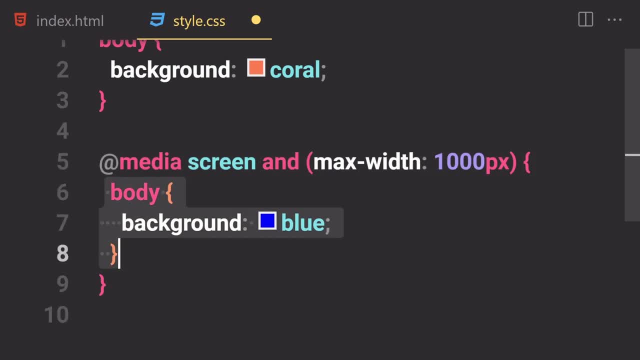 this media query means that we are writing some style like this body. in this case, we are writing some style for the screen size, and that screen size, which maximum width is like thousand pixels knife, is our file. and here you can see, we are now get back to our coral color right here. so where is 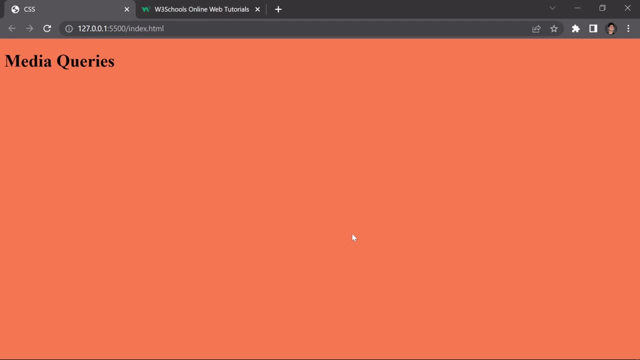 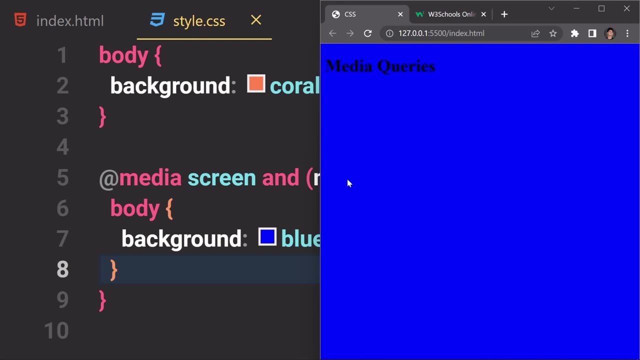 the blue color which we wrote inside this media queries, if you just make our screen size a bit like smaller, like so. so here you can see it: unlock uses their blue color right here. why is that? that's because our current viewport is maximum than 1000 pixels. let me just show you how is that. 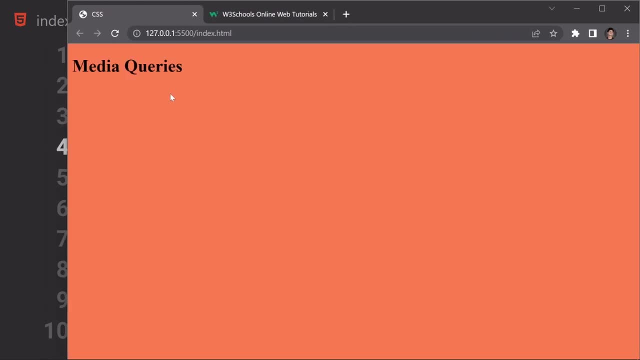 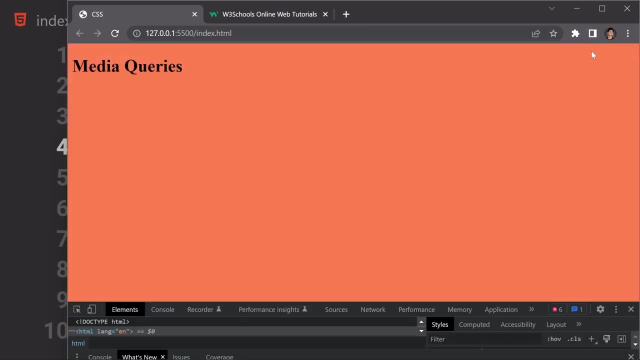 i'm going to make that a bit bigger. so here you can see the log uses that coral color right here. i'm going to right click on that and then just click on this inspect area and i'm going to set that to the bottom and i want you to just focus on this. 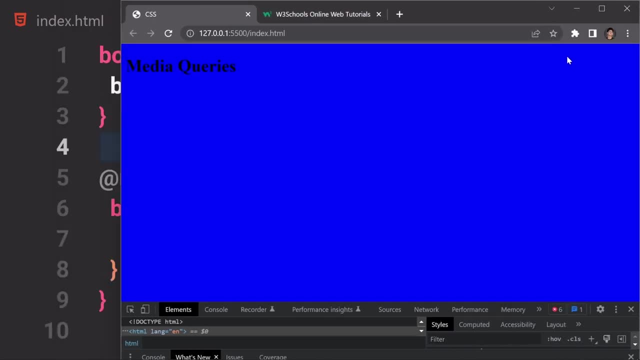 area. so if i just either increase it or decrease it, so here you can see there's screen sizes, and i guess you cannot see that in a recording, but if you're writing this code for yourself, so then you can see it a bit better anyway. so if you just make that a bit bigger, so here you can see, we get like 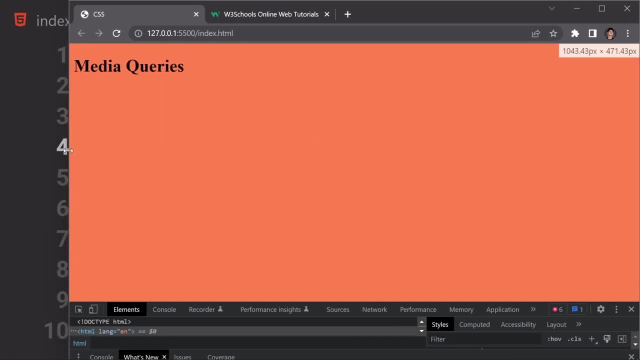 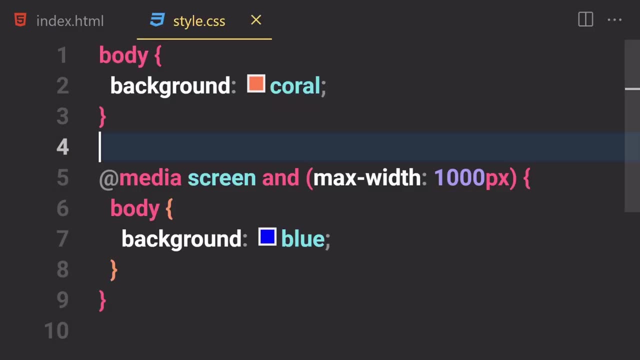 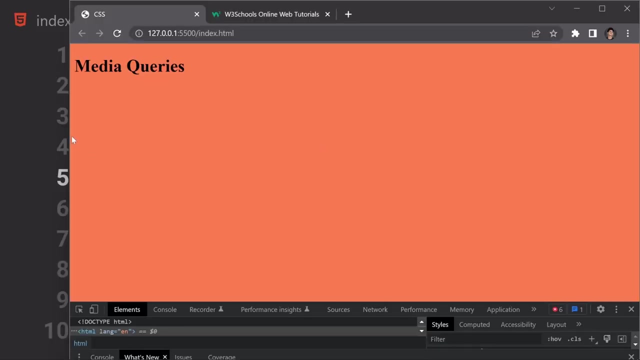 1054 pixel right there. so if you just make it a bit smaller, so here you can see that media query does not match because here we just wrote our media queries. i mean like we want to provide de-styling once our media query hit like a maximum width is like thousand pixel. so if you 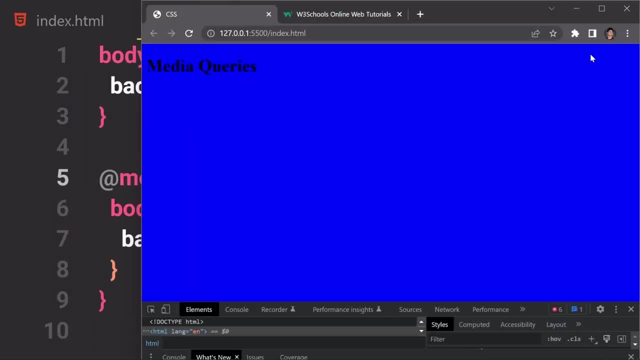 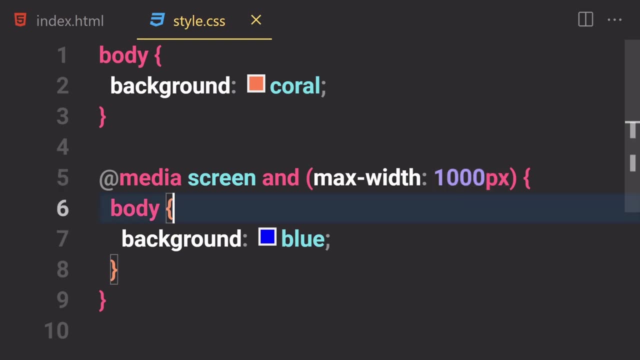 just, uh, make that a bit smaller. so here you can see, like we have like uh, nine thousand and ten, uh, not nine thousand, but nine hundred and ten pixel. so what media query did match. so here you can see, it will now change the color to blue, and you are not just limited to change the body color. 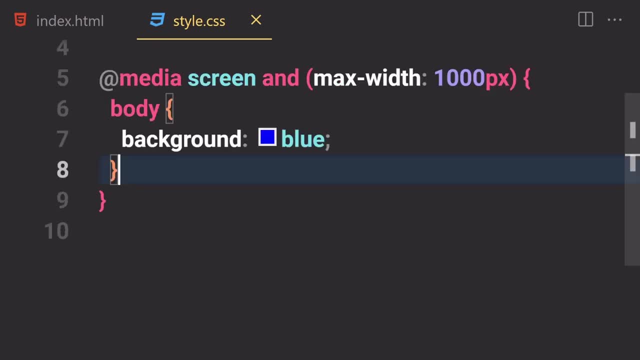 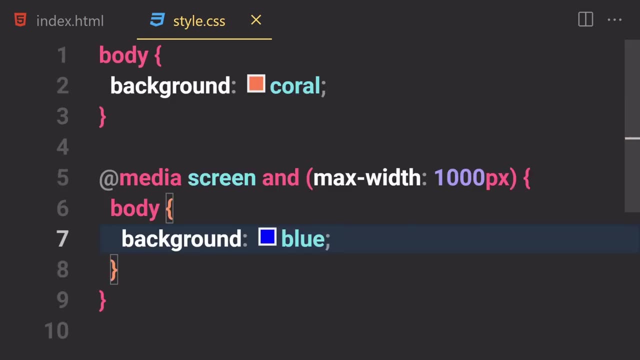 you can do a lot sort of stuff with that, like you can use a display property and the background color, the font sizing, their transformation. you can do a lot sort of stuff with that, like you can use a display property and the background color, the font sizing, their transformation, animation and all kind of that good stuff. 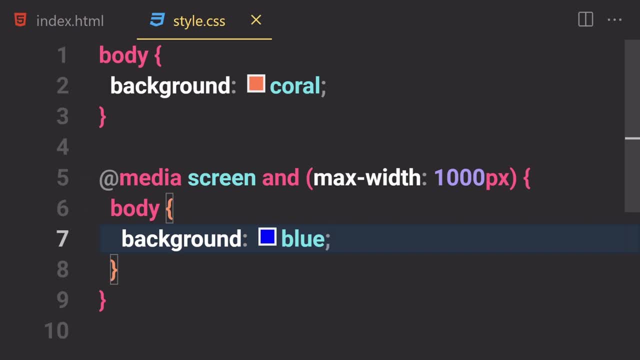 you just learn in this video. so you're not just limited to background color and you're also not just limited to write like a thousand pixel. right here you can write- uh, i don't know, you can write a media query for like 700 pixel if you want to. so now, if you sell a file and we're not getting, 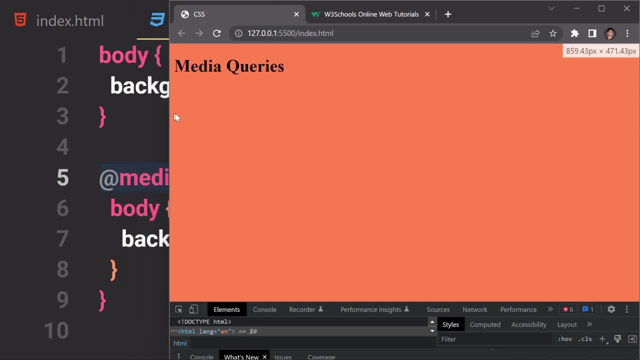 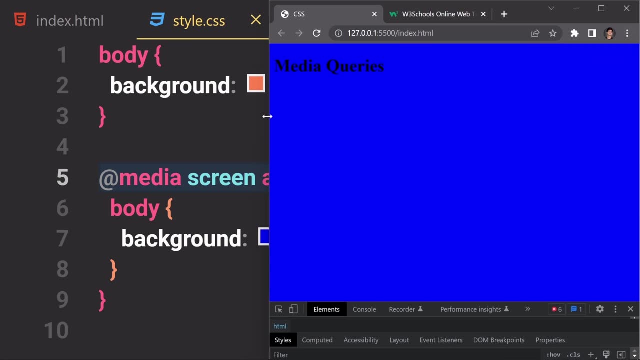 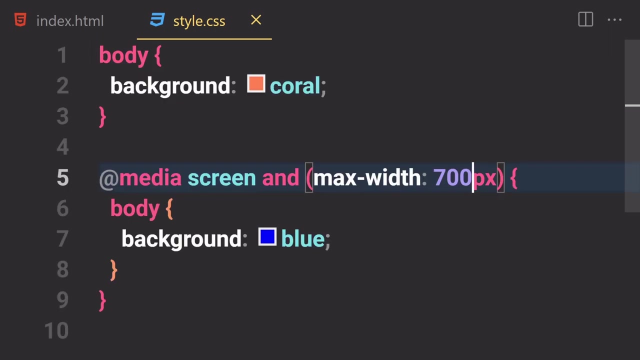 that coral color right here. so if you just make that to 700 pixels, if you hit that media query, okay. so here you can see what maximum width is now like 700 pixel or below that. so here you can see that balloon just gives us that background color of blue right here and we can write different kind. 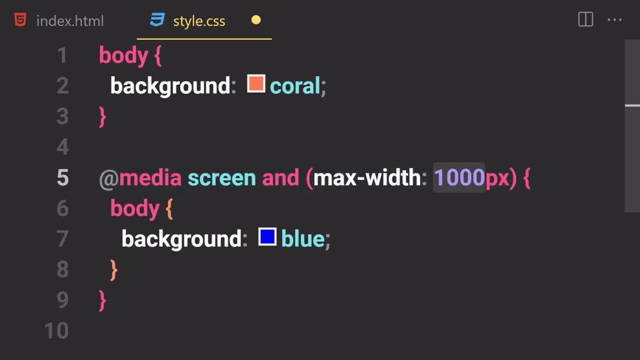 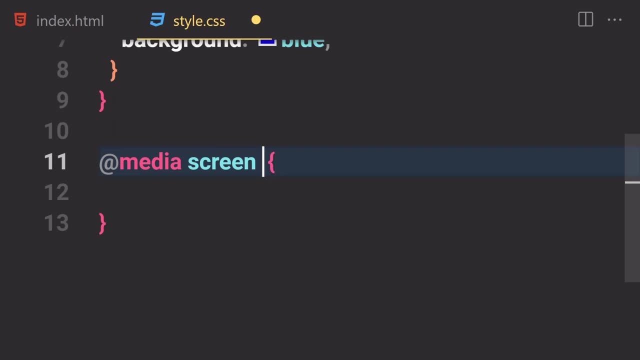 of media queries, if you want to. so i'm going to just change that to like thousand pixel, and now let me just write a new media query. so let me just write a media query for like a different kind of screen size, if you want to. you know what i'm going to do. i'm going to just write a media. 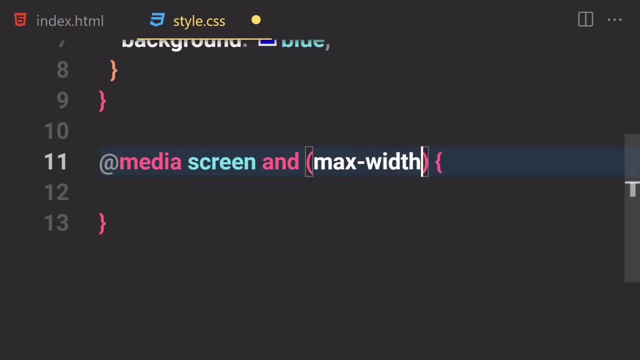 query, for let me just write a max width and you can also write a minwith if you want. so max width just means like the maximum width and min width just simply means like the minimum width, with okay, so we can just write like i don't know, 700 pixel in here and now let's just get our body. 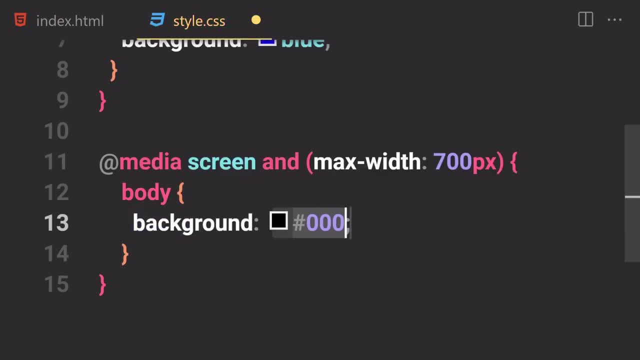 and you know what? in this case, i'm going to change the color to be like a steel blue and i'm going to also change the font size, uh, to be like i don't know font size, to be, uh, five frame would be fine, so you can see the reference if you save a file and here you can see it on now. first of all, change: 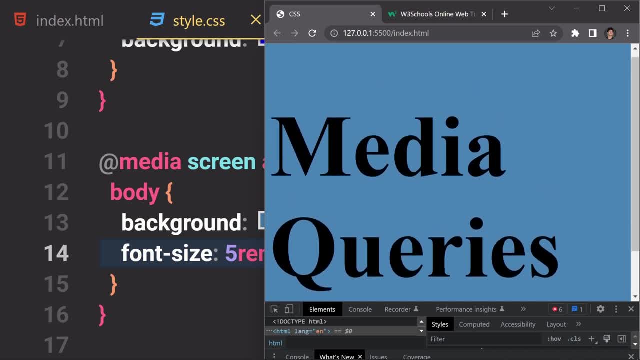 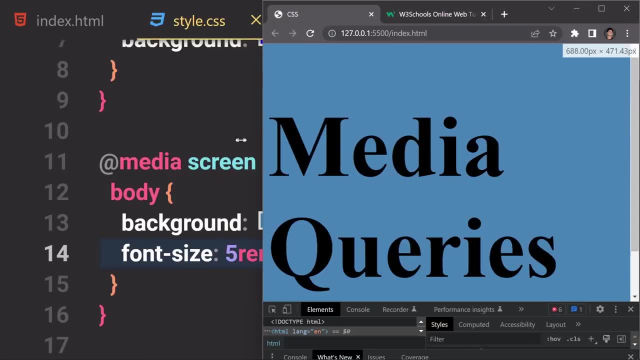 the background color to be that steel blue and it will also increase the font size to be five frames right here. that's because our media query match. so we are now getting this styling. so if you just make that a bit smaller, and here you can see, the font size is normal and the background color is. 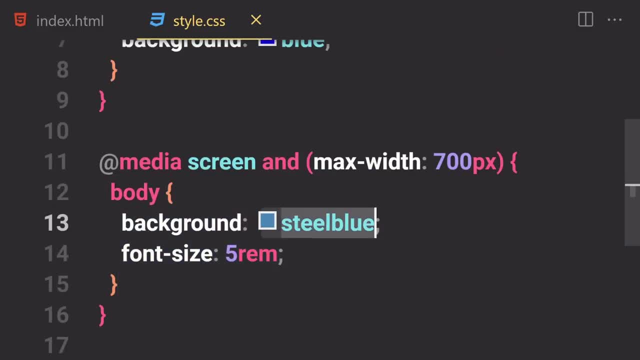 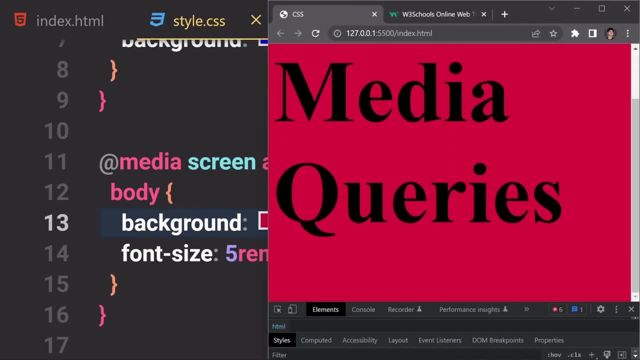 changed to totally blue, and you know what these colors are, kind of the same. so i'm going to just change that to crimson and a few side of that, and now, if you just make that a bit smaller, so here you can see now the difference. okay, so this is how you can provide different kind of style and 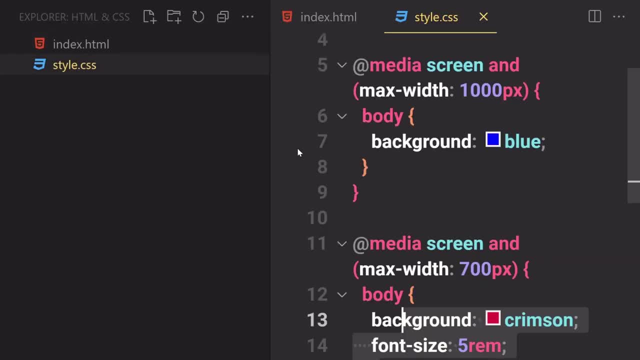 different kind of media queries. i'm going to just zoom out a bit so you guys can see everything a bit clearer, and then i'm going to change the font size to be like a steel blue. and i'm going to change the font size to be like a steel blue. and this one is the first media query. this one is the. 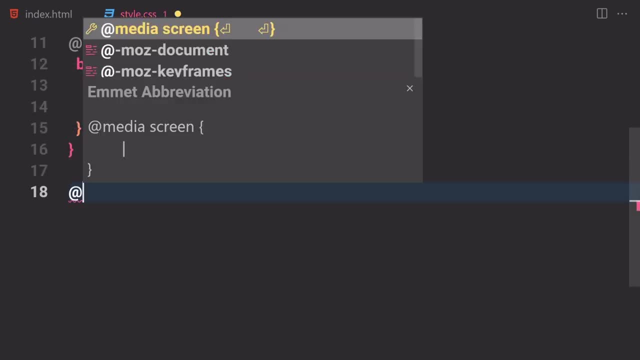 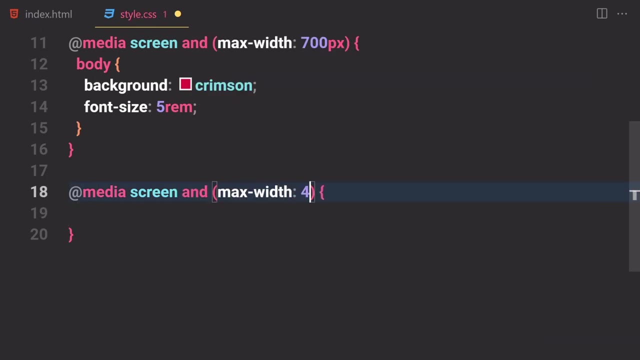 second, media query, and we can just go below there. if you want to just write a media in here for a screen size and let's just write and symbol, and max width will be like, i don't know, maybe for 400 pixel, but you know what, 400 is just a little bit smaller. i'm going to just go with a 500 pixel. 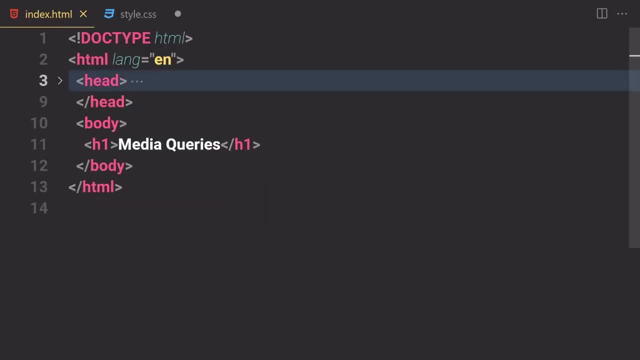 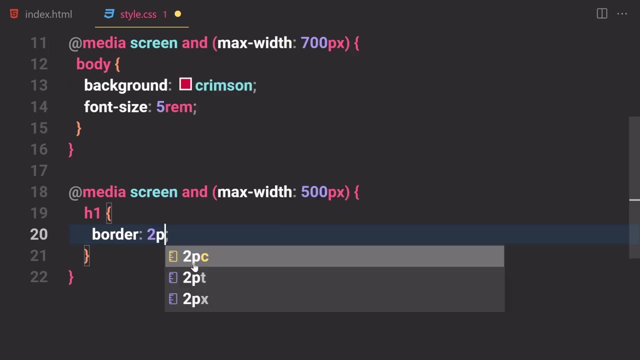 and what i'm going to do. i'm going to just, um, you know what i'm going to just write: select this h1. right now, i'm going to select that h1 and i'm going to just provide, like, a border of two pixels, or not two pixels, but four pixel dotted, and then i don't know um, what should i give a color to be? 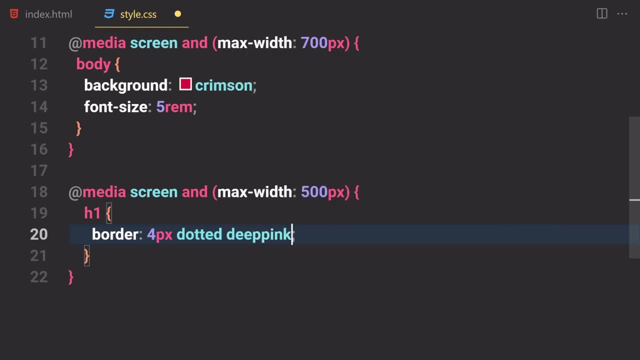 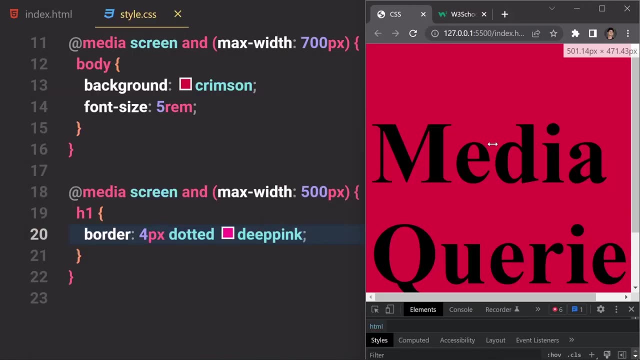 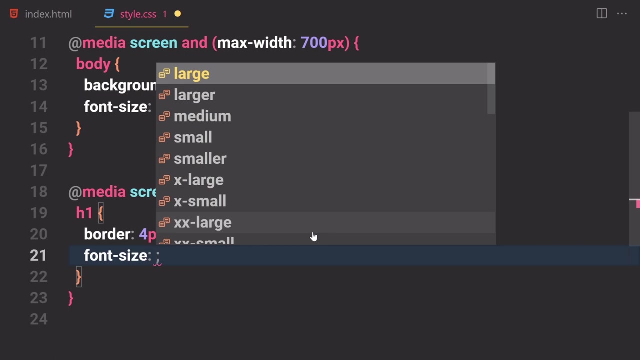 uh, i don't know, golden would be fine, or deep pink would be fine in this case. if you save that and if you just make the screen size a bit smaller, okay, so it's not showing up in here, that's because our screen size is small. uh, huge, let's just write a font size of maybe one rim. 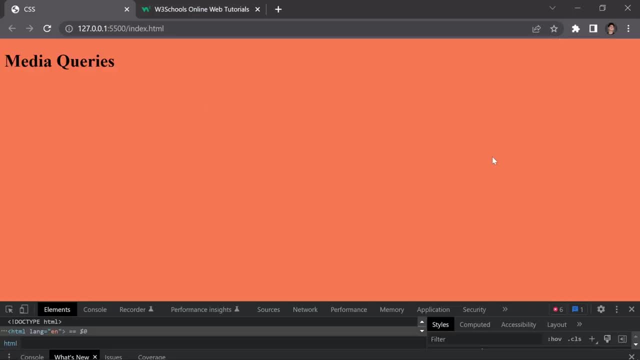 and several file. and now let me just make that a bit bigger, okay, and let's just click on these three dots, or you know what? we are not going to be clicking on these three dots, we are going to be clicking on this kind of a screen, so i'm going to just click. 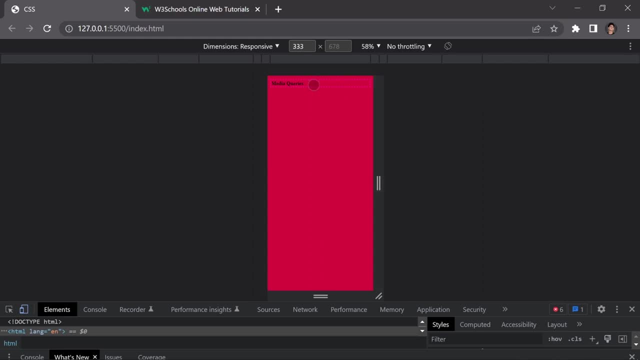 on that, make it a bit smaller, and here you can. okay, you cannot see that difference. i'm going to change that to maybe blue, and if you save that, and here you can see now where h1 have the border of four pixel dotted, uh, blue, uh, kind of a border right here, here you can see the difference and i 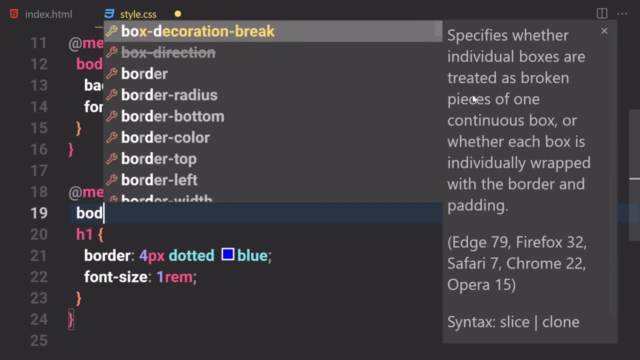 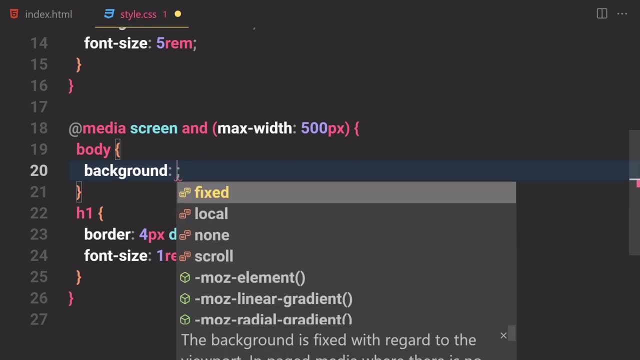 cannot see that. you know what? i'm going to change the background to be something else. let's just write a body and change the background to be something else. like i don't know, you know, i'm going to go with a totally white color. why not? so i'm going to just go with a. 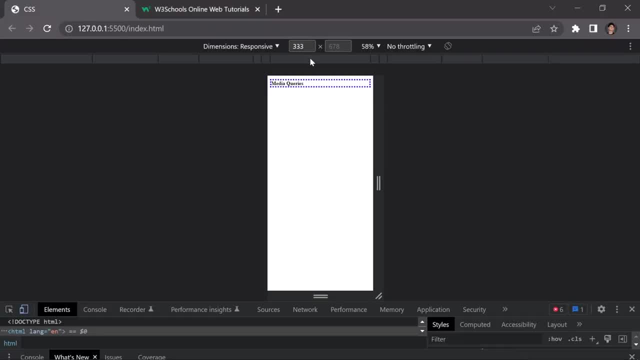 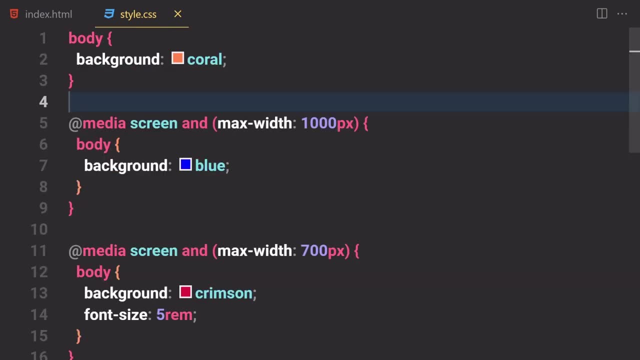 totally white colored cell file and now you can see the difference right here. okay, so this is how you can provide a lot of different kind of media queries and, by the way, we are not totally done with the media create. there's a lot of things you can do by using a media queries, but this was just 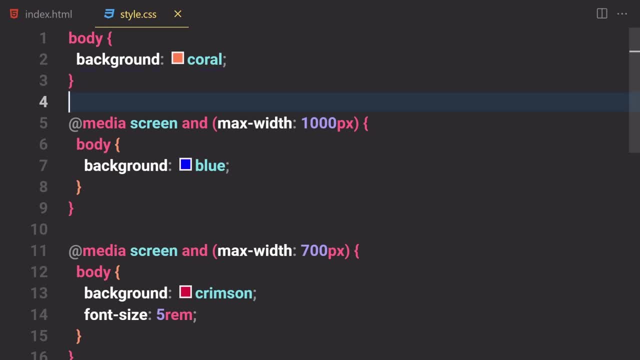 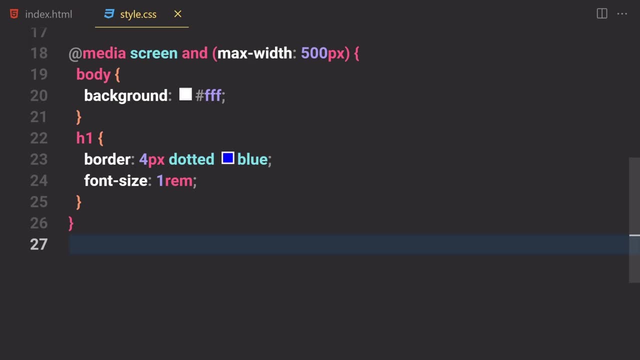 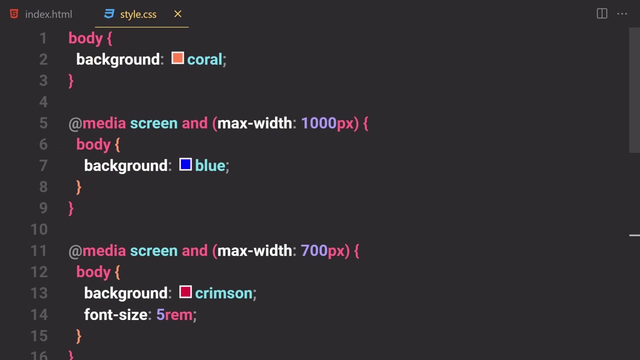 a test so that you can work on your projects. and i'm going to make a huge uh guide on media queries. but i cannot promise you that right now, but i'm not sure. but by the time you are watching this video i guess i will already provide the video. but if i didn't provide it already, so then you. 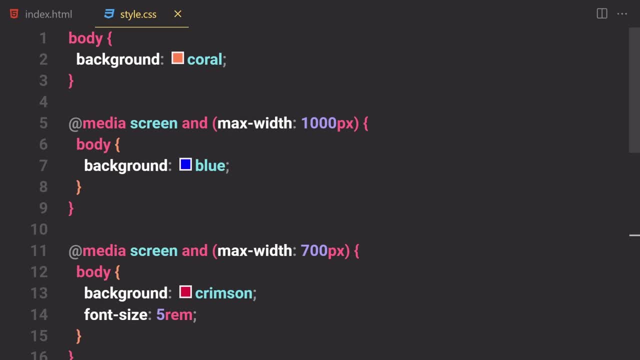 have to wait for the a little bit anyway. so we are not totally done with the media queries and now let's jump into building a projects. or you know what? first of all, we have to learn um, what do we call? it emits. or you know, we are not going to be providing any image. i'm not going to. 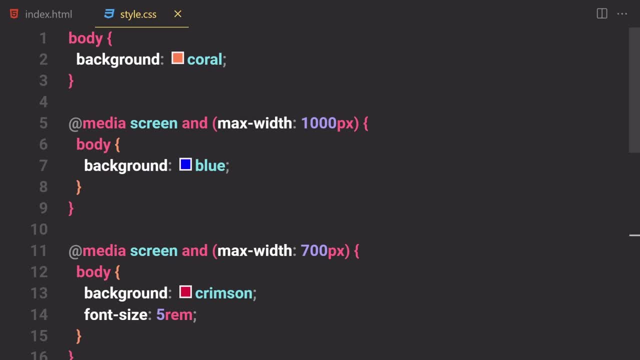 provide any image. i'm not sure i will, or i will not if the next topics was on about emits. so congratulations, you got a bonus. emits are not related to html and css. it's kind of a other topic to learn. if you didn't see the image section after this, well then, you have to check out my video. i 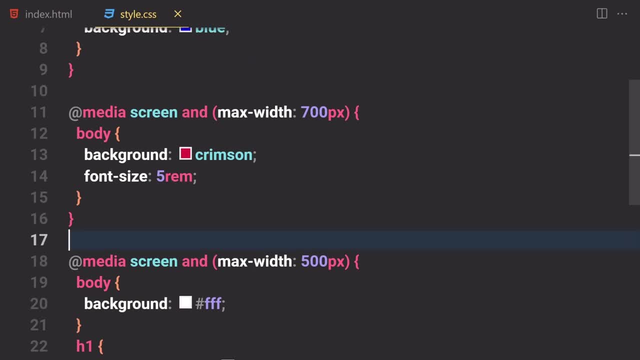 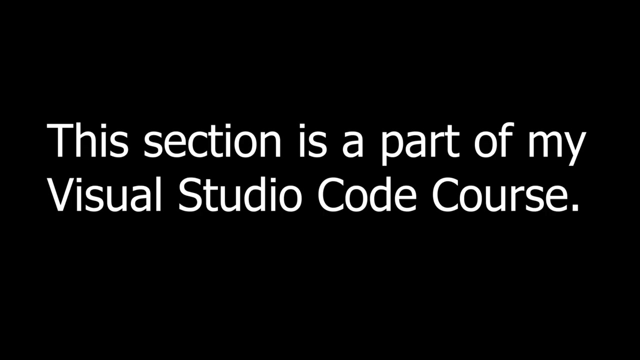 have entire- like i don't know- half an hour radio on emits. you can learn a lot crazy stuff about emits. you can check it out if you want to, uh, and i guess i'm gonna go into the projects, so i'll see you in the projects. i don't want to waste your time and mine as well. all right, so now that we 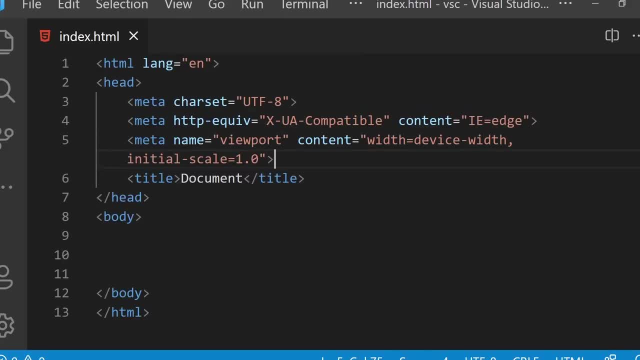 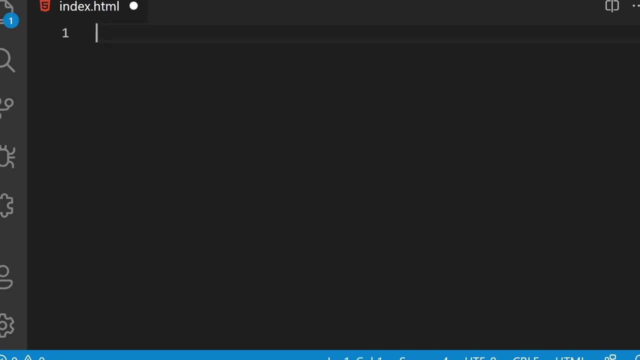 learned a lot of shortcuts in visual story quarters, so the next thing which you have to learn is something called emits in visual story quarters. so what in the world are emits? first of all, i'm going to remove everything from here. i'm going to make this screen size a bit bigger so you guys can. 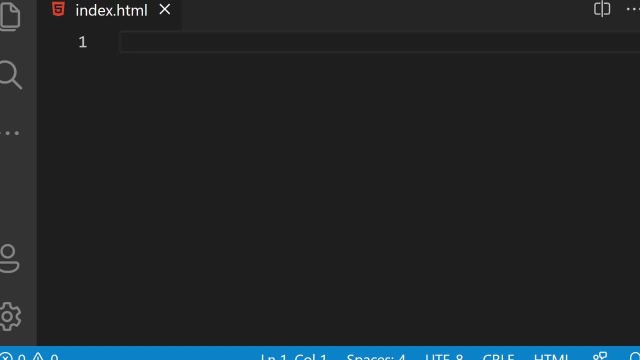 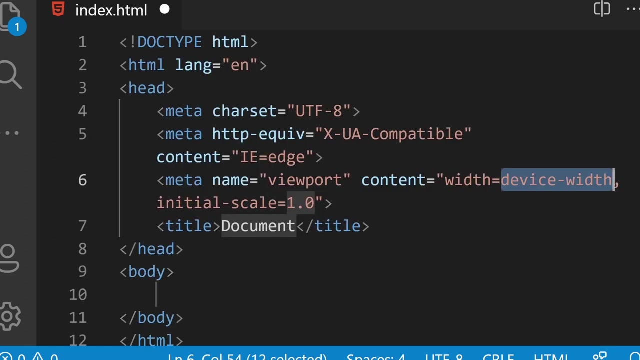 get better. so what in the world are emits in visual story coders? so emits are abbreviated code that follow the same convention as html and css and we can use that convention like. we can just write, like i don't know, explanation mark and then hit tab and it will just generate. 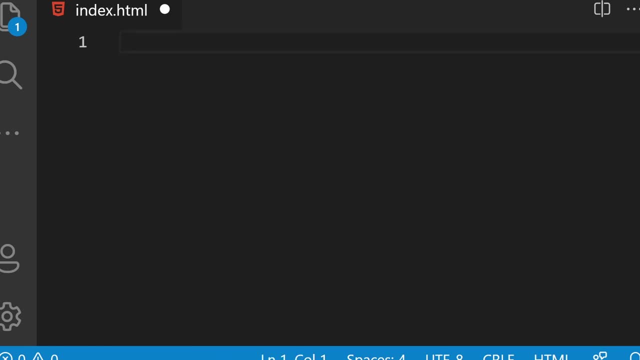 this stuff for us, so it allows us to write our code very, very quickly. so in this section we are going to be learning a lot about emits and i'm going to show you different kind of emits in html. so let's just start from the first one, which is a boilerplate emits. so what is a boilerplate emits? 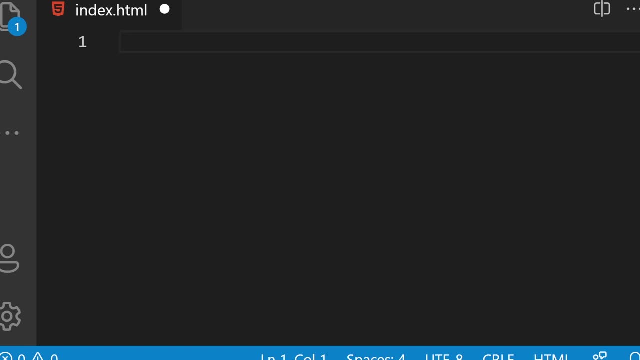 first of all, if you want to get html structure in visual story quarters so that you don't have to write like html, like html: opening tag then the head, opening tag and closing tag, then the- uh, i don't know- like a title opening tag and closing tag, then the body, so you don't have to waste your. 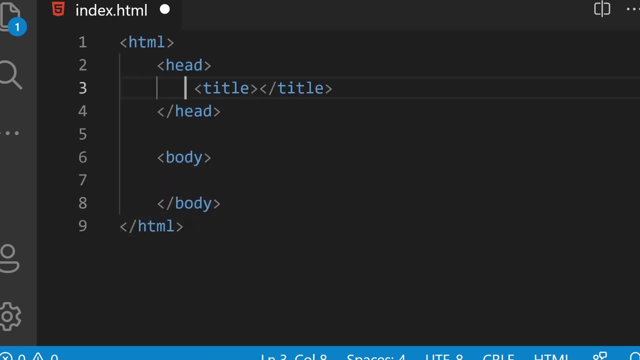 time in there and, by the way, i also forgot to mention like you can also provide a metadata css file, but it will waste a lot of your time. so what's the best way? well, we can use something called image, so so we can get the same result by using our image. so the first way is to just write. 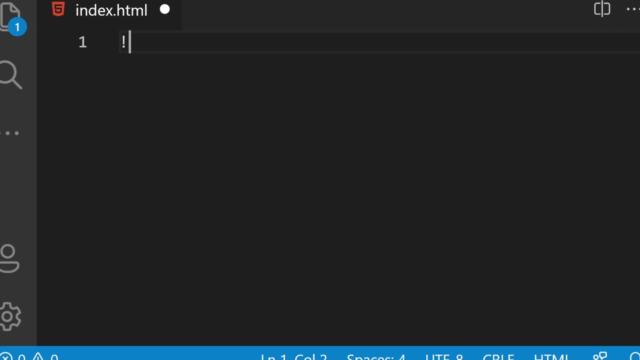 explanation mark and hit tabs. so how can you get this explanation mark? i want you to just hold shift and hit one, so it will now give you that explanation mark right here. so if you are hitting tab and it's not working, so then you can hold control and hit space, and then you can hit enter. 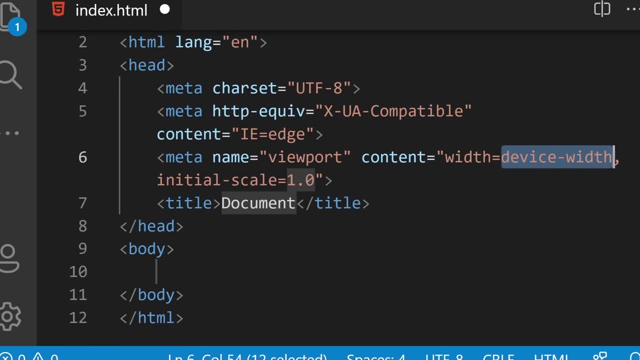 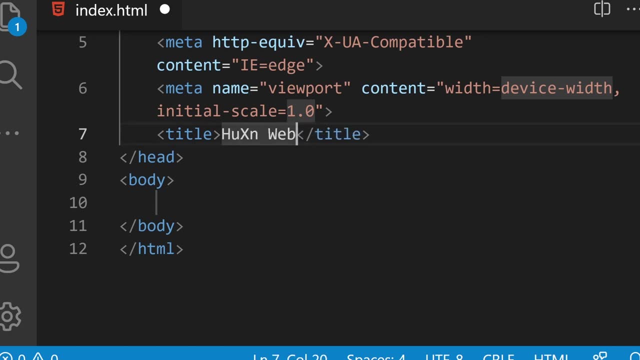 and it will give you that html structure right here, and then you can hit tab and hit tab one more time and you can change the title to like i don't know my own name, like huzzan web dev, and then you can hit tab and then you can write your code like: so okay, so this is the first way we can. 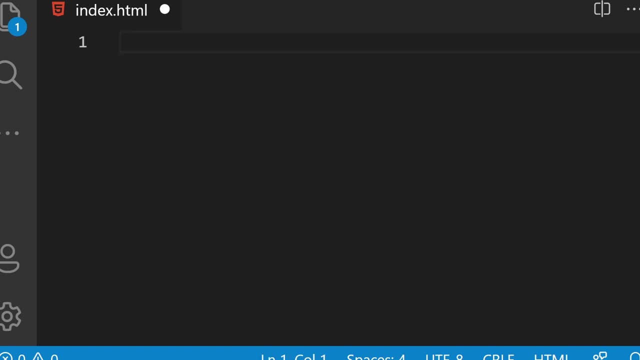 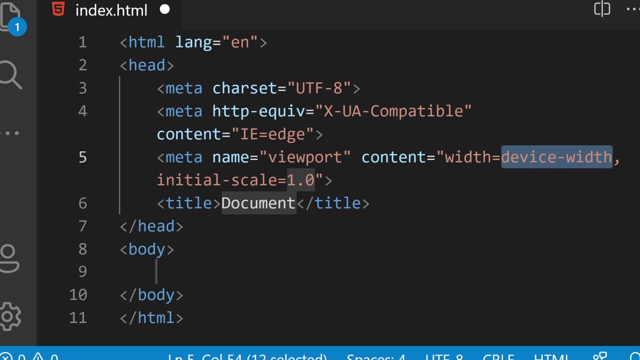 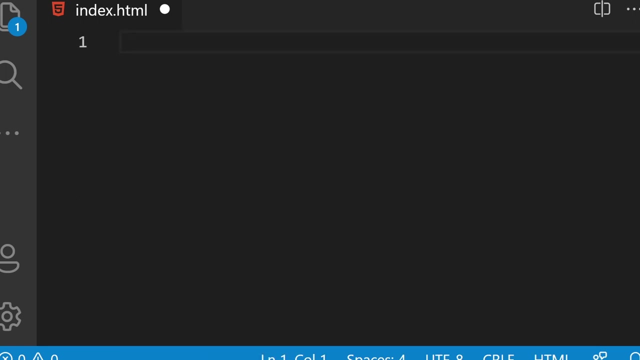 get or html structure. so what's the next way? the next way is to just write doc for doc type html. now, if i hit tab and here you can see, it will now also gives us that same html structure right here. okay, so both of them will work the same. so you can either choose like doc or you can also. 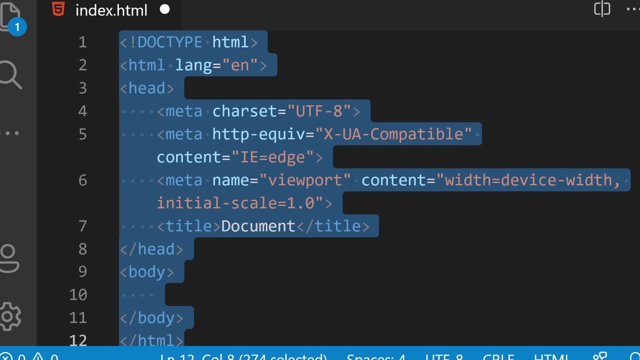 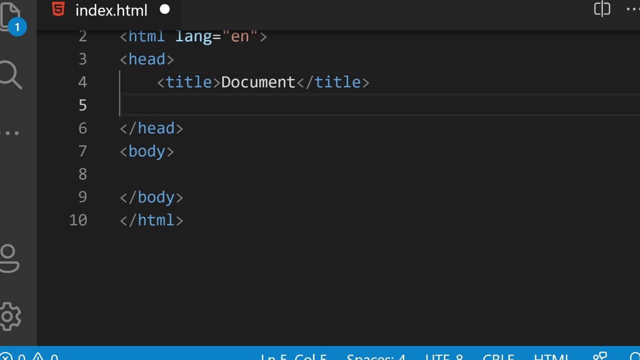 just choose like explanation mark, and both of them will work the same. all right, so let me just remove these metadata from here, because i don't need it right here. okay, so what else do we have to do? so now, let me just show you a shortcut for linking with css. so instead of writing like link and then 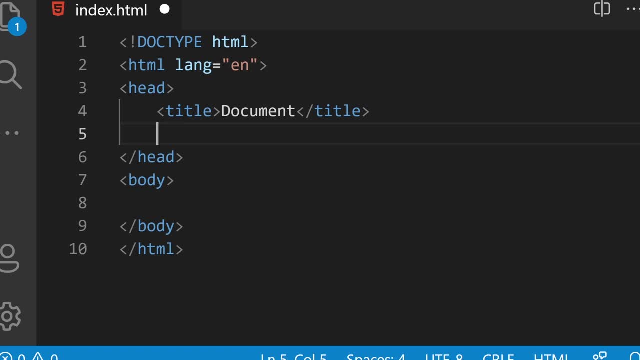 rel, stylesheet and stuff like that. you can use image, so you just have to write like l i, n, k and then hit tab. so here you can see, it will now gives us that link and it will also gives us that relationship with stylesheet, and we have href. 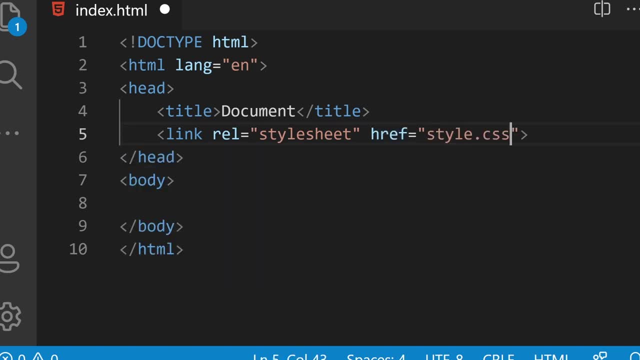 and we can just hit control and space and then we can link it with any file we want. okay, so that was the first. so you just have to write link and hit tab and here you can see it will just fill it out for you, i mean like it will just cue the boilerplate for you, and you can also choose like: 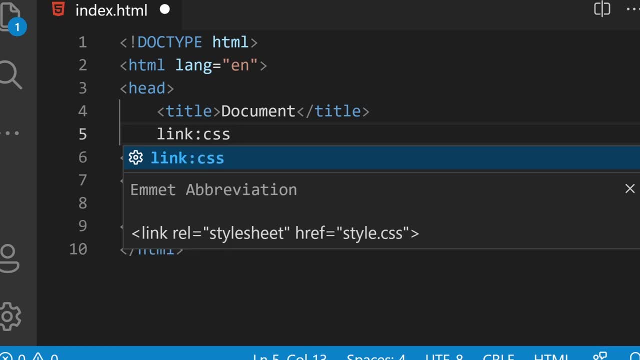 link, and then colon and then css. and now if you hit tab, and here you can see, it will also fill it up with this stylecss file as well. and now here, if i just send my file, so everything will work. but if my file name is changed to like: 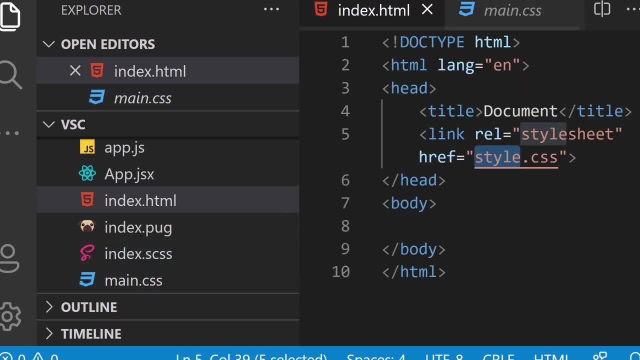 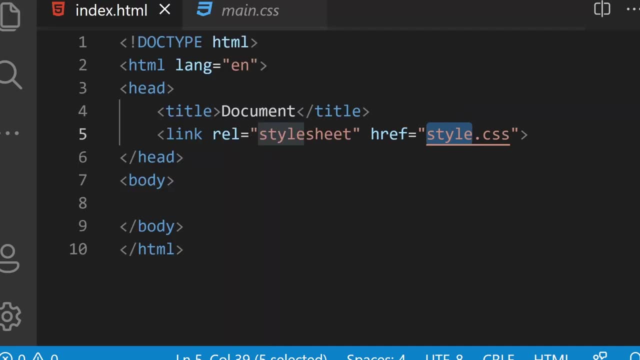 something else like main, and if i hit enter, so then it will not work. it will give you that stylecss but it will not work. like it will not choose this maincss by default. so i want you to notice that one as well. so i'm going to set that to style one more time and there we go. okay, so that was. 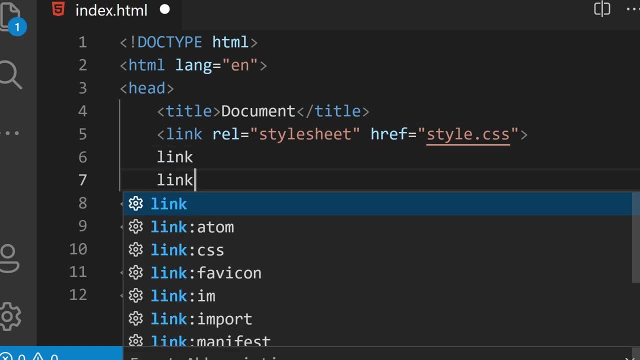 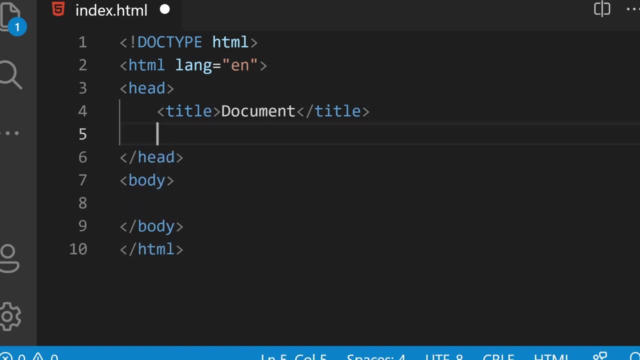 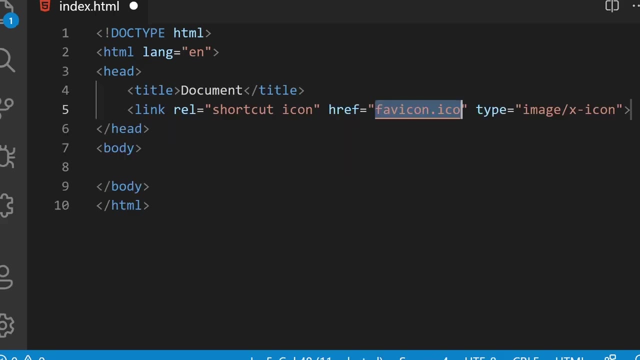 it about a link and also the link, colon, css. and now, if you want to, i'll link it with facebook account, like if you want to provide some sort of a favicon for your project, so you can also just write link and then colon and then favicon. okay, and now if you hit tab, and here you can see it. 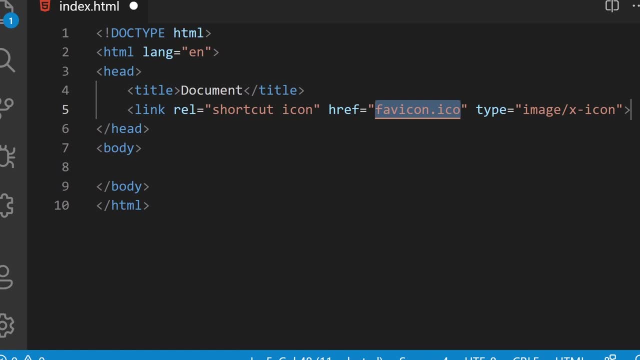 will not give you all of this stuff which you need for a favicon. so we have a link, then we have a relationship with the shortcut icon, and then we have icon, and then we have type, which will be now set to image, and x icon. so this is how it looks like and you can just provide your. uh, what do you? 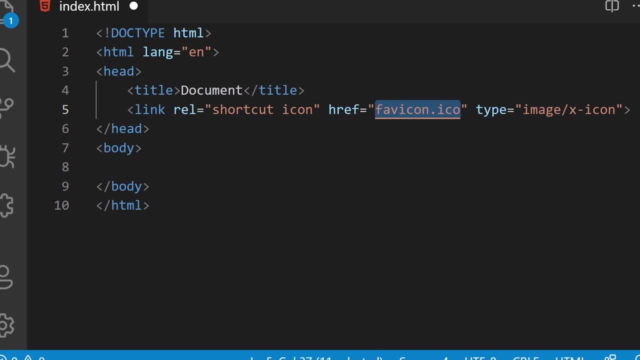 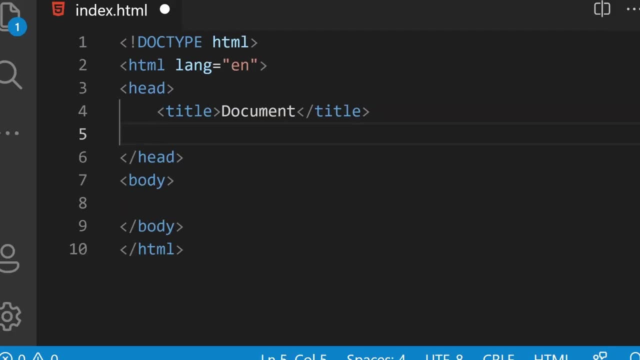 call it. you can provide your favicon link right here and then you can also add a link to your. i don't have any favicon links, so sorry, i can't show you that right now. i'm going to remove it from now anyways. so that was how you can link it with your css, and now let's just learn about. 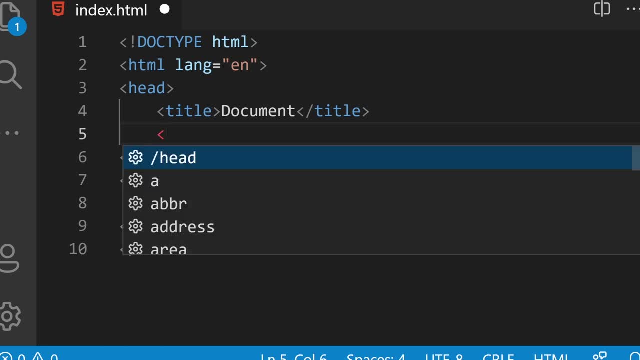 styling. so now, if you want to provide internal style so you don't have to write like less than sign and then close it right here, and we just recorded it will also help you with that. but you can also use image for that. you just have to write style and hit tab okay, so here you. 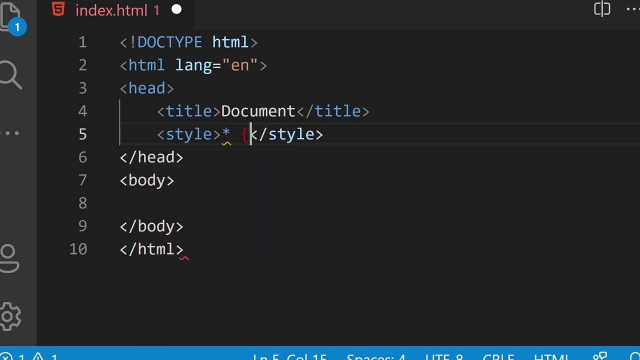 can see, it will just auto complete it for you. then you can choose anything you want, and then you can provide your own styling to it. okay, so this is how you can also provide internal styling, and now let's just learn about how we can link it with our javascript file so we can. 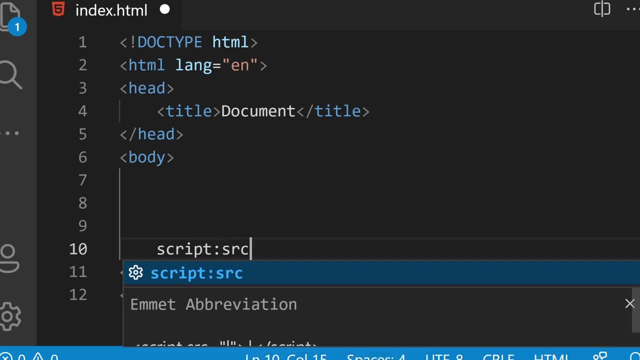 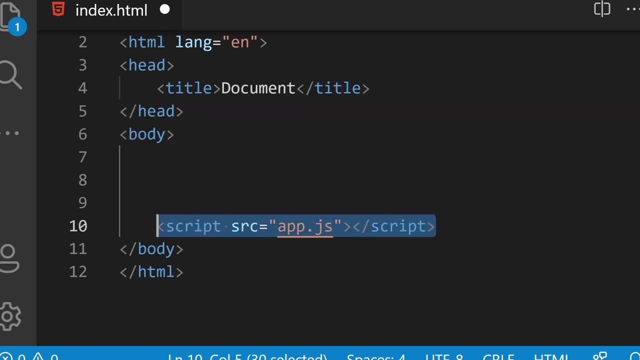 just use like script and then colon src for source, and if you hit tab and here you can see, then we can use control space and then we can choose our javascript file right here. okay, so that was just a basics of emerge. so i'm going to remove all of that from here and now let's just learn about the. 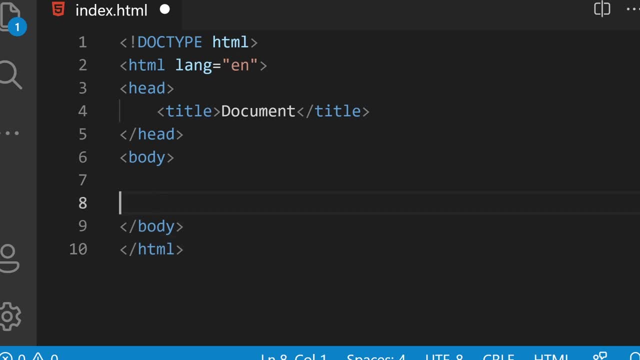 image. so we just learned about a boilerplate image, so now let's just learn about basic image. so instead of just writing like uh, listen, sign, and then h1, and then it will just close it up for you, and then also instead of just writing like list and sign and section and all of that, and then then 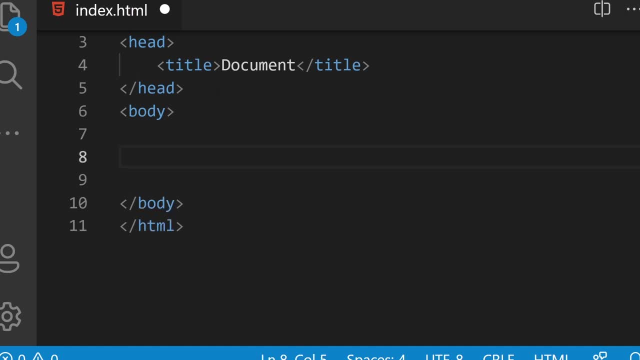 you have to close it. so instead of doing all of that, you can just use your image. so just write h1 and hit tab, and now, here you can see, it will now just fill it out for you. okay, so you can use h2, h3, 3n, hit tab, h4 and hit tab, h5, and hit tab h6 and hit tab, and here you can see, it will just fill. 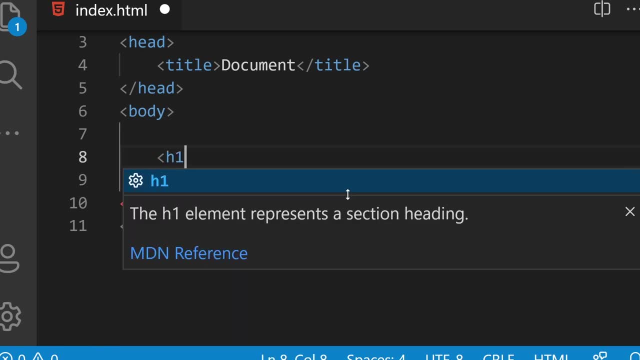 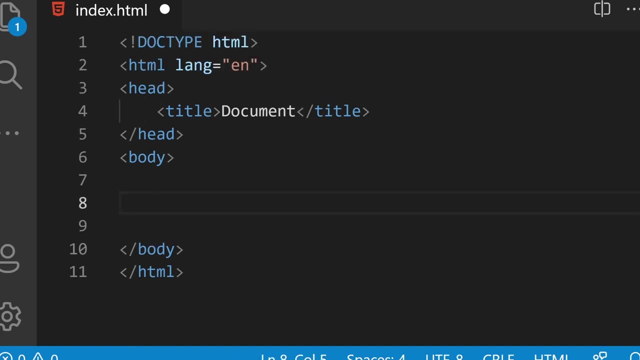 it out for you. you don't have to write like list and sign and then h1 and then close it right here. you don't have to do any of that stuff. okay, you are now using emit and emit will give you a super power and you can also just omit by just writing like a whole section. you can also omit that too. 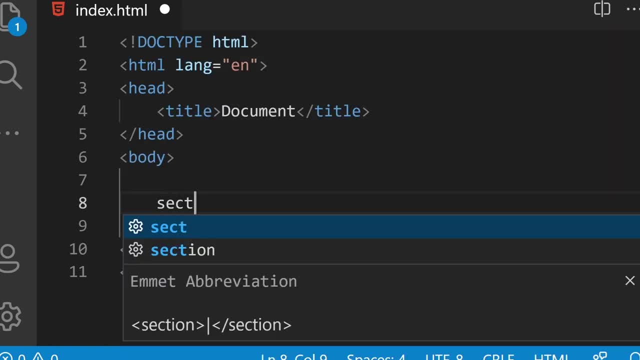 just like sec and not sec, but sect. and now, if you hit tab- and now, here you can see- it will just auto complete it for you. and then- and you can also just write hdr and then hit tab, and here you can see, it will now give us header and you can also just write art and hit tab, and it will. 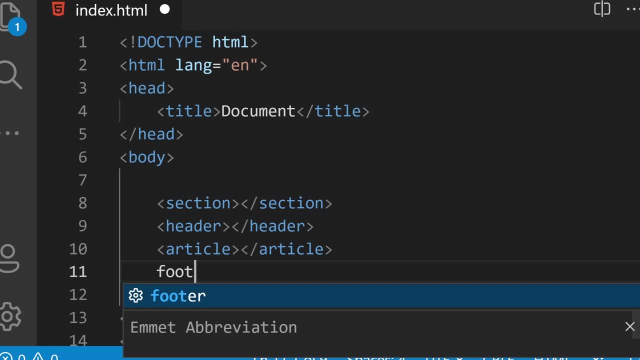 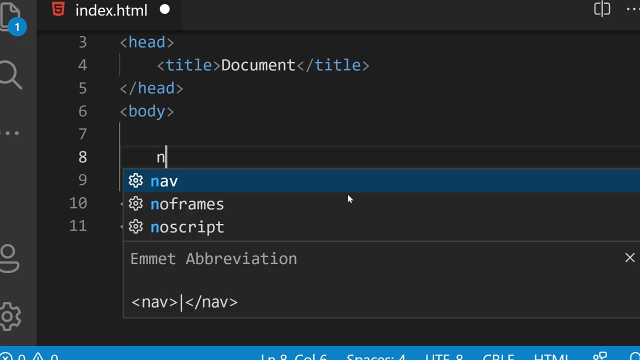 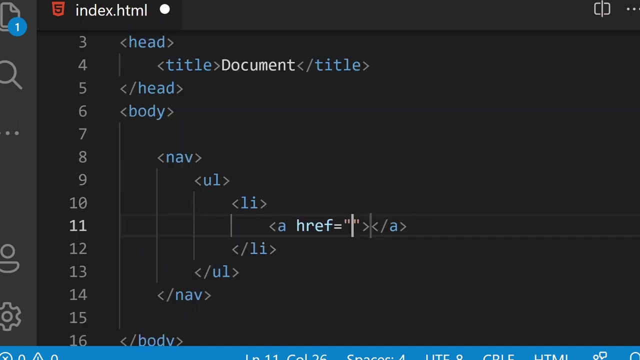 just give you article and you can also just write like f, double o, t and hit tab, and here you can see, it will also give you the same results. so you can also just write like um, nav, nav is a symbol, so you just have right now and there will work, then u and hit tab, li, hit tab anchor tag, hit tab and. 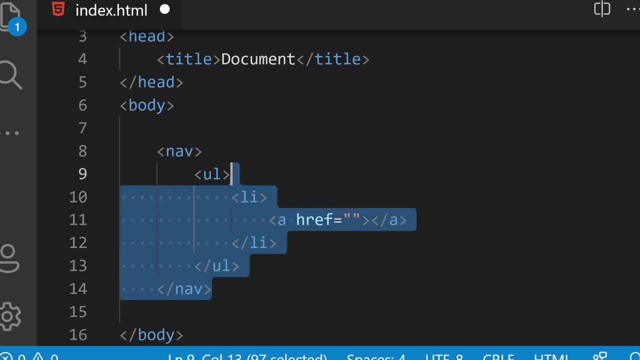 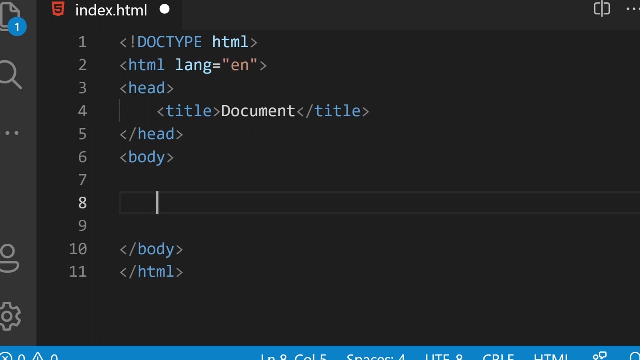 here you can see. you just have to write the first word and hit tab. it will just auto complete it for you. okay, so that was just a basics of emit. so now let's just learn about uh, css- selector emit. so what do i mean by that? so if you previously work with css, so you already know how id works, how the 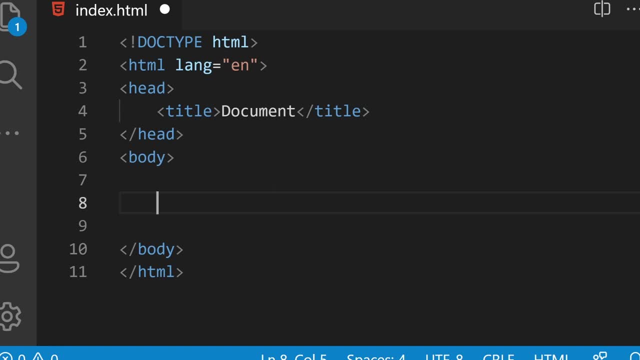 classes work and how you can select that. so if i ask you, like, how can you select, uh, this section by id in css? well, you would just say, like you will just go to your style sheet and you would just provide a pound symbol and what was that? the section? so you will just write a section and then 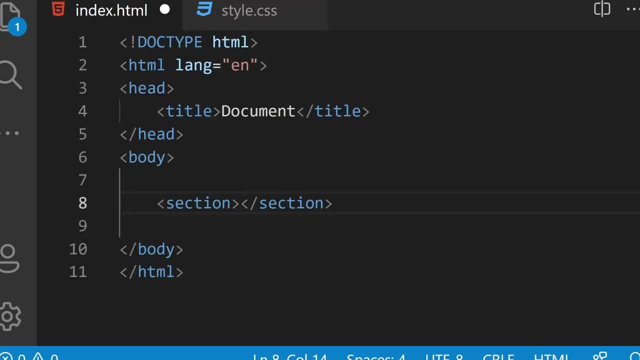 you can provide different kind of style shirt. so if you already work with the css, so this is how you can use that, like, first of all, you just write a pound symbol and then the section name, and then you're going to specify your colors and styling. okay, so now if you want to provide id to something, 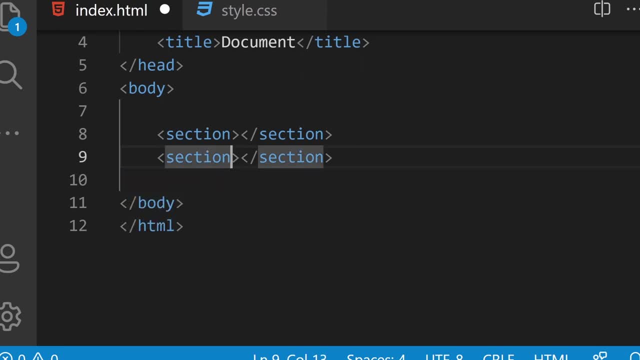 so you don't have to just write like section, then close it, then hit space and then provide id and then just give them some sort of id. so it will waste a lot of your time. so instead you can just write the element name like section or s, e, c, s, e, c, t, and then write a. 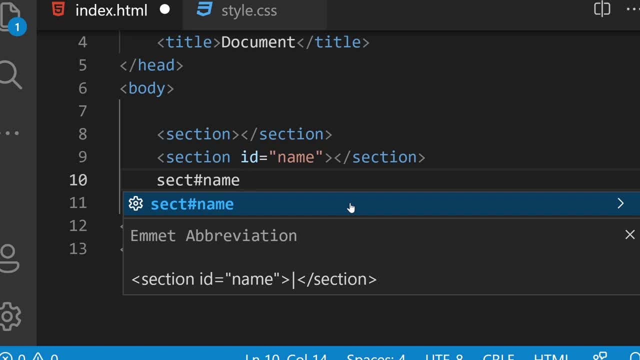 pound symbol and then you can just give a name of whatever you want and hit tab and first of all it will just auto complete your section or whatever the element name was, and it will also give you that id and then it will also fill it out with the name you specified right here. so if you don't want, 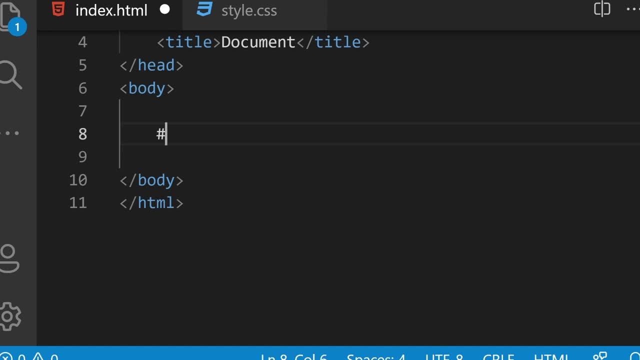 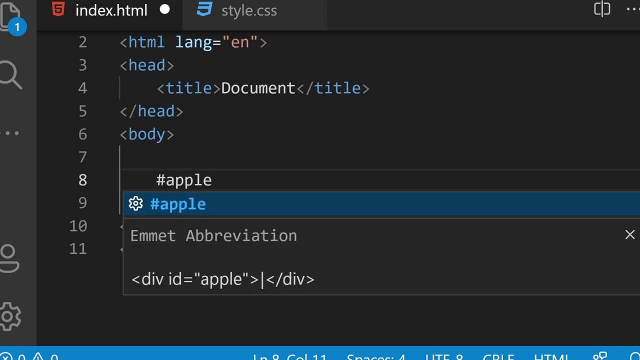 to provide any elements whatsoever, so you can also just use a pound symbol. i mean like, yeah, pound, you have any kind of id name you want, like i don't know, apple would be fine. and if i hit tab and here you can see, it will by default gives us a div and it will fill it out with the id of apple. 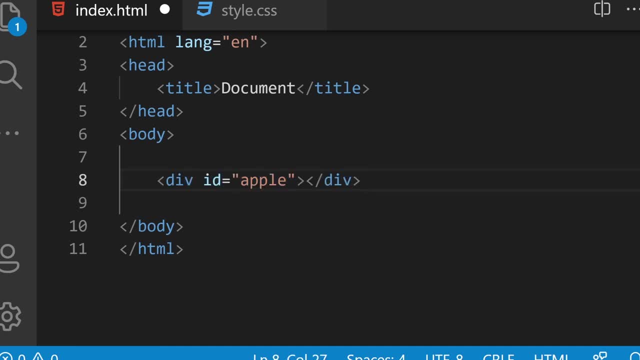 okay, so this is how we can provide ids to something. and now, if i ask you to select this article, how can you select this article? uh, in css, by using a class. so you would say like: first of all we have to give them some sort of a cluster like cls name, and then, if you want to select it in css, so first, 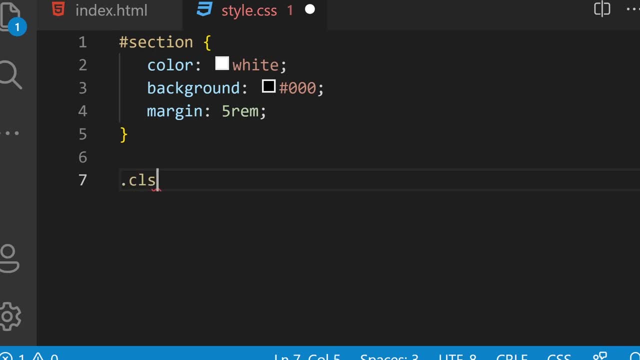 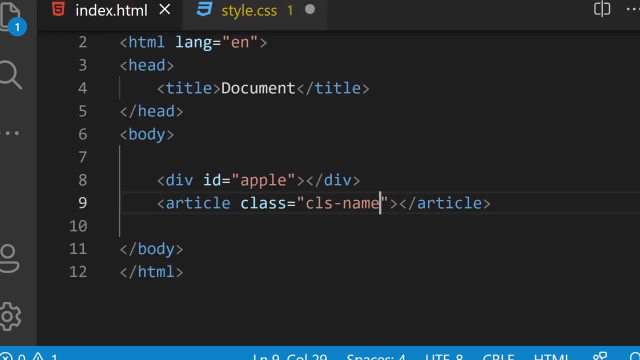 you just write a period or dot, whatever you want to call it, and then the class name you, you select that and then you can specify your styling and whatsoever right here. so the same will go to the html, so you don't have to write article and then just write like article and then write a space. 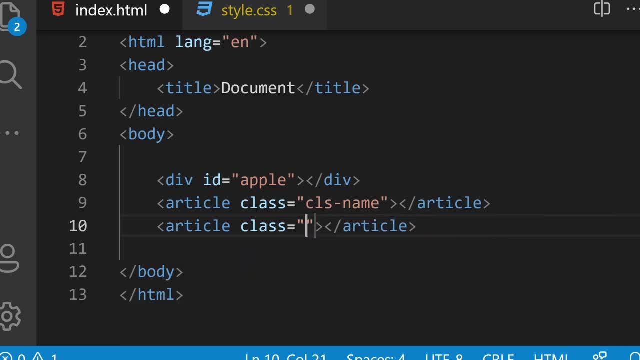 and then just write a class and then you can give them whatever the class name is. so instead of doing all of that- like instead of writing article, then class and then, yeah, spacing as well. so instead of doing all of that, you just have to write, like art, and then write a period and then you can give. 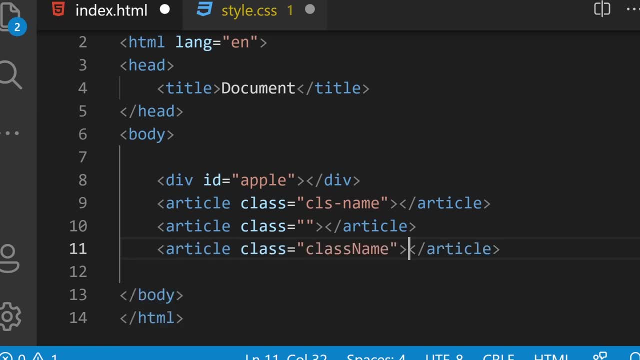 any kind of class name you want and then hit tab and here you can see it will just fill it out as article. it will give you the class and the class name will be filled out with whatever you provide right here. so you can also just give my own name and here you can see it will just fill it out for. 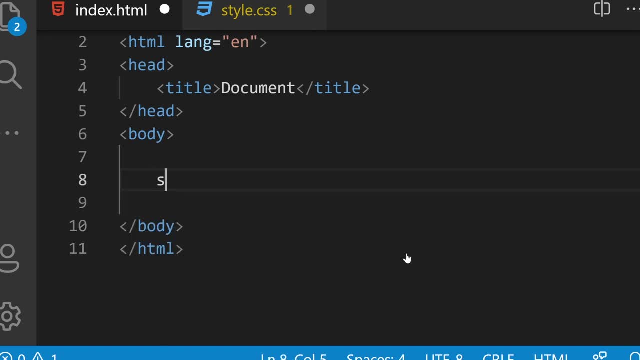 you and you're not just limited to write article, but you can just write like section and then just give me some sort of a class name and it will just give you that class name. you can write a navigation with a class of like i don't know- logo. you can also just write ul of. 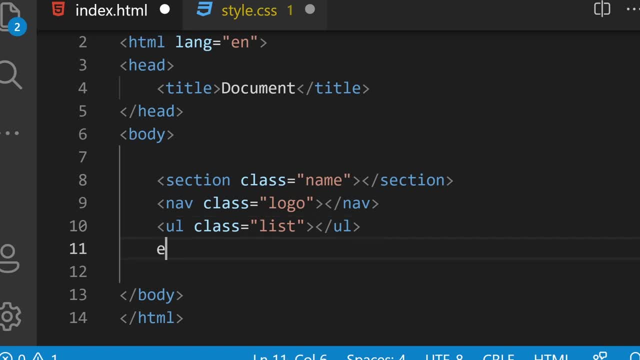 list and it will just fill it out for you. you just have to write first of all the element name and then the period and then the class name. okay, so this is the basic syntax of it. so i'm going to remove all of that from here. so now that we learn about how you can select something by id and how, 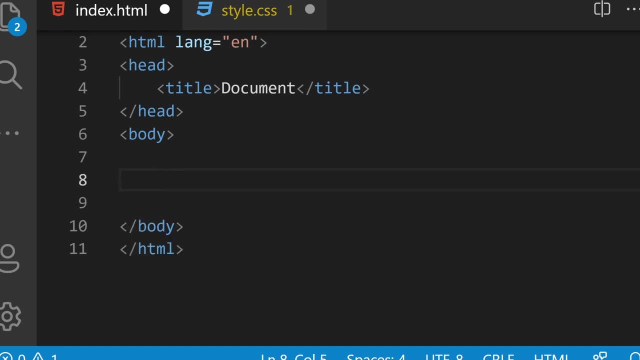 you can select something by classes, and we already learned about how you can select something by the element name, so you just have to write h1 and boom. okay, so that was that. now let's just learn about nesting and emirates. so what do i mean by nesting? 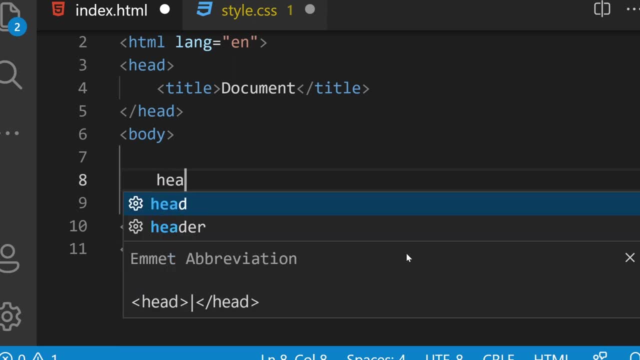 so in some situation you would have a lot of nesting, like you would have a header and inside this header you would have some sort of a navigation and inside that navigation you would have a ul. inside that ul you would have a li. inside that li you will have, or your anchor tag. 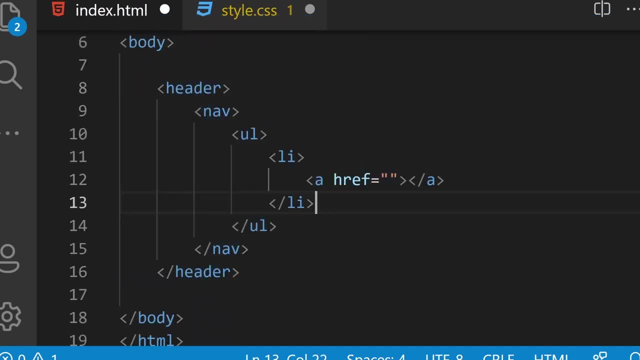 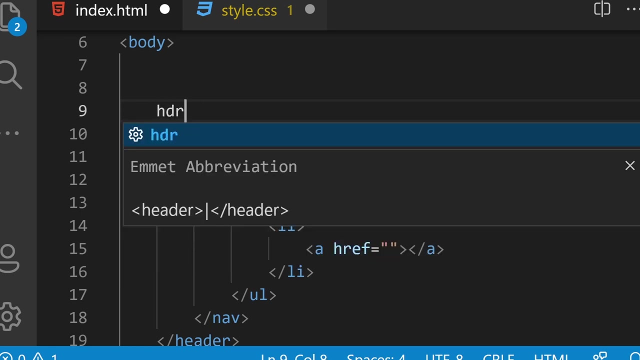 and this structure will look like this right here: so instead of writing like header, then navigation, then ul, then li, then anchor tag, instead of writing all of that, so for that you can use emirates. so how can you write that? well, so you just have to write header, or you can also shorten it to like hdr, if you want to. 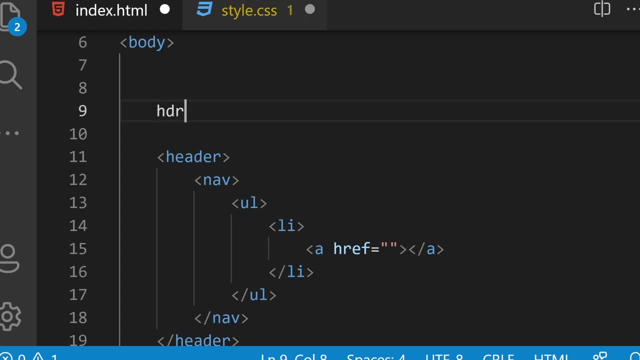 and let's just see what was the next one. the next one was nav. so if you want to provide nested element inside that header, so you just write a greater than sign and then you can specify another element. so in this case i'm going to just write nav. and now, if you want to provide another one, 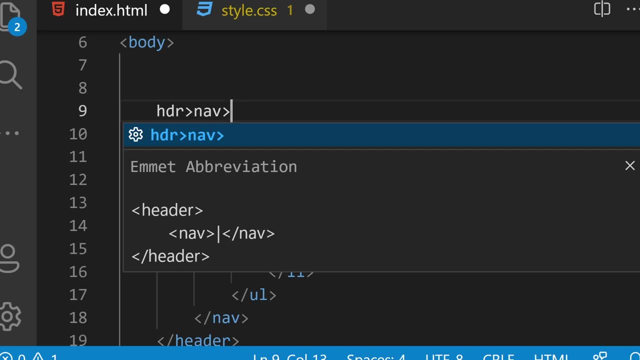 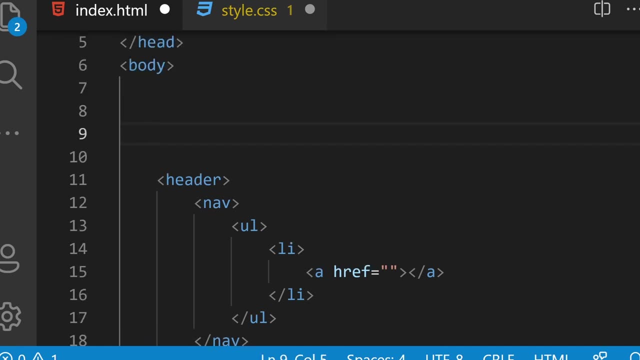 so you can also just hit greater than sign and then you can provide another one, and then you can provide another one like ul. let me just give you a quick example of that, and then i'm going to write that header and stuff like that. so first of all let me just write hdr and inside this hdr, if i want. 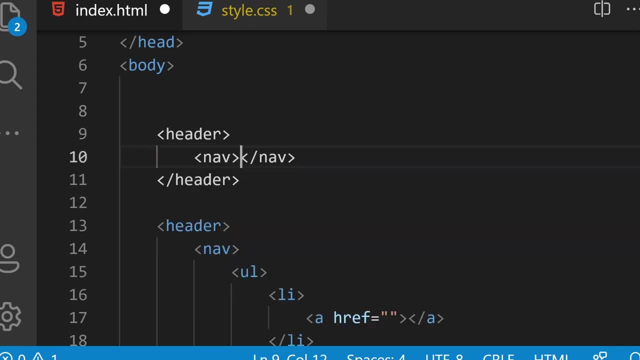 a nav. so i'm going to just write a greater than sign and then nav and if i hit tab and here you can see, it will now give us header opening tag, header closing tag and nav opening tag and nav closing tag. so this is how you can work with that. so i'm going to remove that and i'm going to write: 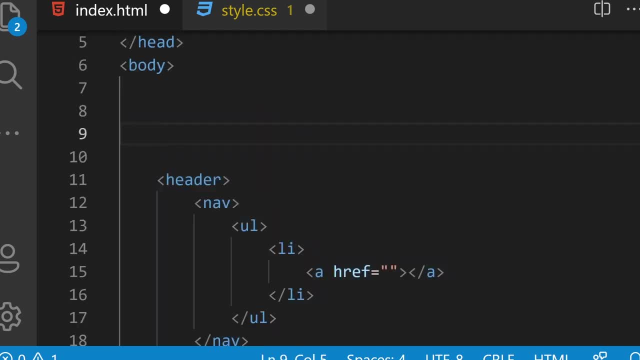 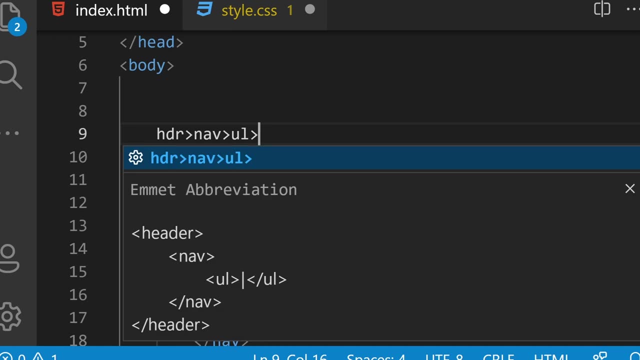 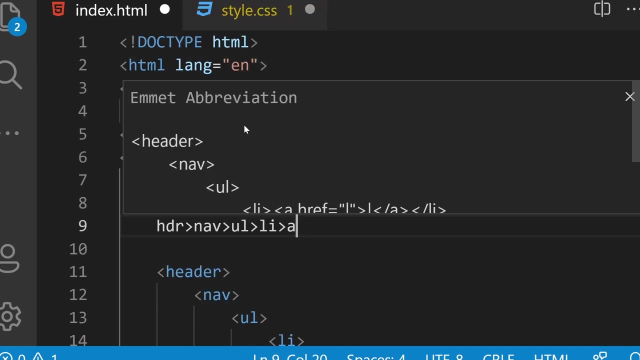 an image for all of these codings. so what do i have to do? i'm going to write hdr for header inside this header. i want navigation, inside that navigation, i want my ul, inside that ul, i want my li, and inside this li i want my anchor tag. okay, so now, here you can see the preview of that coding. 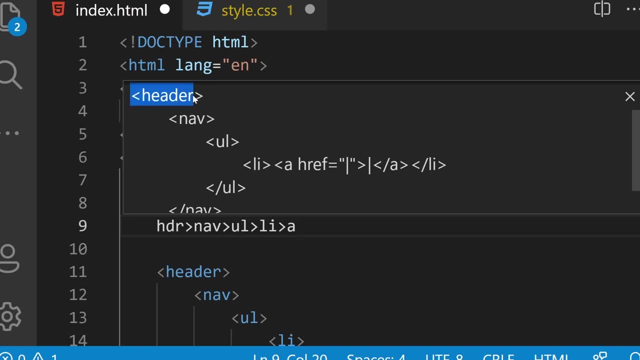 right here, so if i just make it a bit smaller. so first of all we have a header, then we have our navigation, then we have our ul and inside this ul we have our li and inside this li we just have one anchor tag right here and now. if i hit control space and hit, either click on it or 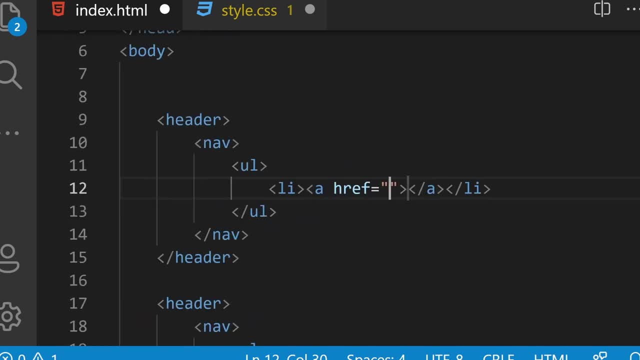 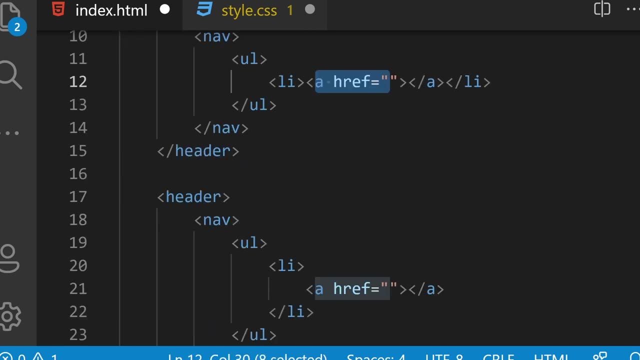 hit tab and here you can see, it will now give us the same result, like this one. so first of all we have our header, then we have our navigation, then we have our ul, then li and then anchor tag. okay, so did. you saw how simple that was. you don't have to write complex things, you just have to write hdr. 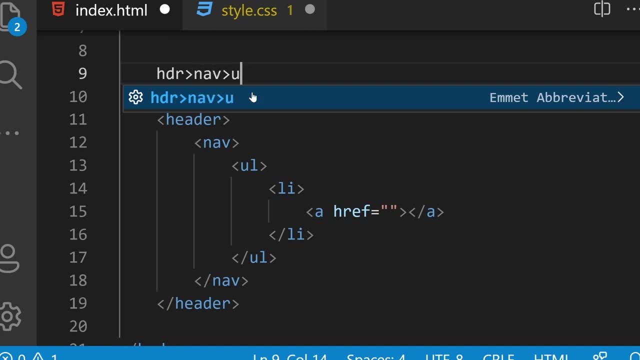 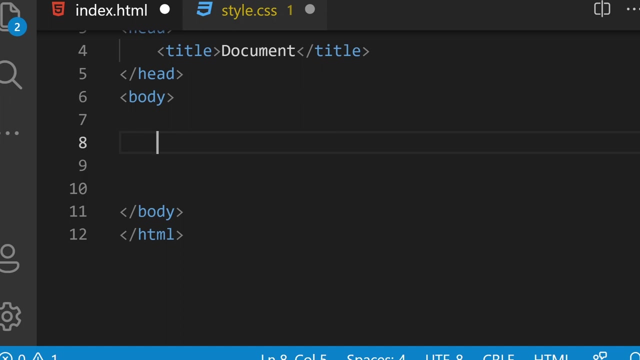 and then greater than sign and nested element, then nested element, one more time, and so on and so forth. so that was about nesting. let me just remove this coding from here and now. let's just learn about a multiply. if you want to repeat some code like a lot of time in html. so instead of writing like: uh, let me just 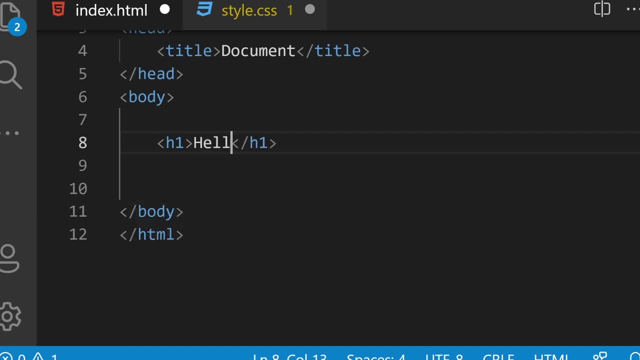 give you example of h1. so instead of writing like h1 of hello, you already know, like, if you want to duplicate this, so you can use a few shortcuts, or if you don't want to use the shortcuts, so you can just hit ctrl c and then ctrl v, so it will just pass it right here a lot of times, so it will waste. 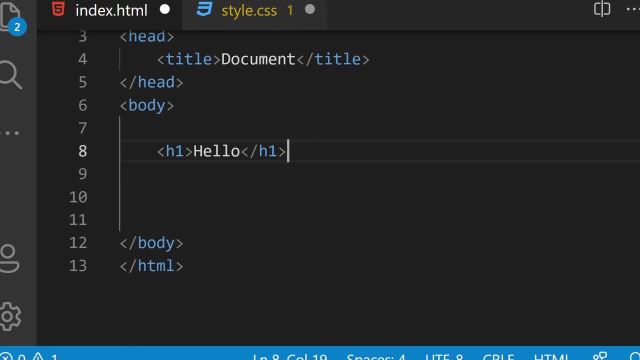 a lot of our time. so instead of doing all of that, you can also use that same shortcut like art, and then shift and down arrow, so it will also duplicate it for you. but instead of doing all of that, you can just use an invert, so you just have fried h1, like the element name, and then the opening curly brace and then the closing. 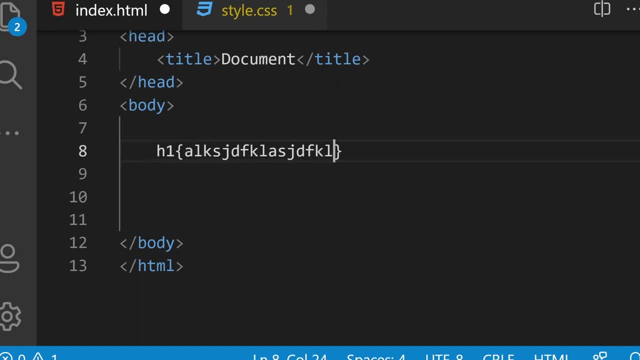 curly brace and inside these curly braces we are going to be writing our text. so anything we write inside there, it will be your text. so i'm going to just write hello. and now, if you want this h1, inside this h1 we have a hello. if i want this result to be like i don't know, to render like 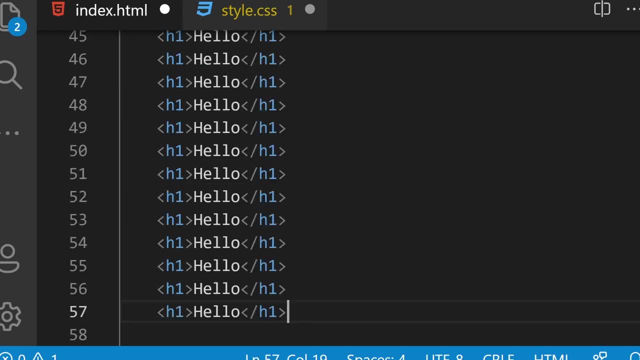 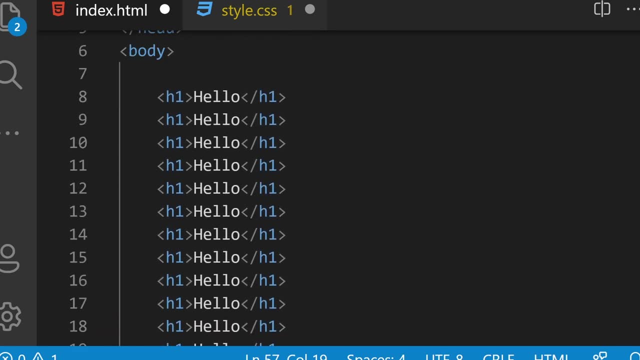 50 percent. so if i just write 50 and now, if i hit tab, now here you can see, we have h1 with the text of hello 50 right here. so now, here you can see, if i just cut it from here, i'm going to remove everything and i'm going to pass it right here. 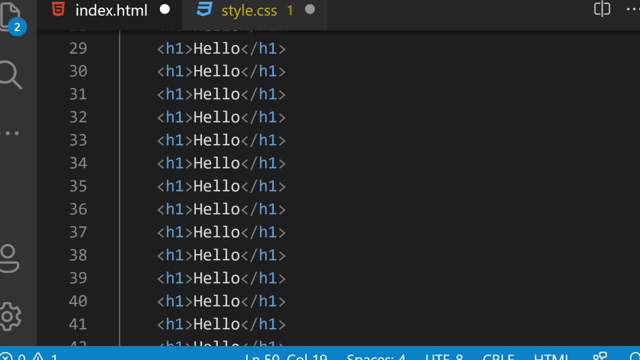 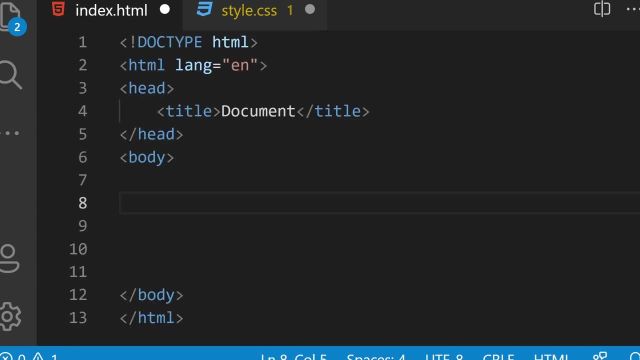 and now, here you can see, we have this h1 from 1 through uh 50 right here. so did you saw how powerful that was. i'm going to remove these h1s from here. we can also just write like: let me just give you example of uh ul allies very quickly. so if you want something to repeat like a lot of time, 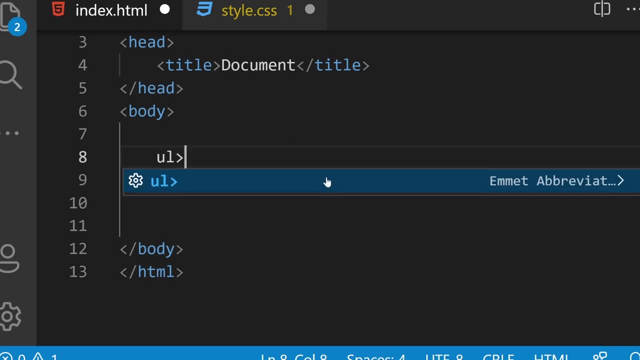 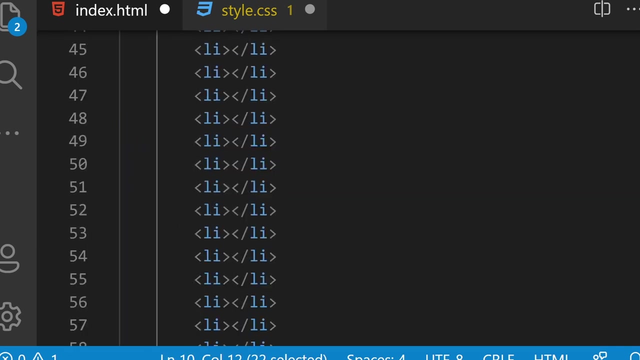 so let's suppose we have like ul inside this ul i have li right here and i want this ali to be like 50. so if i just write 50 and hit tab, so here you can see, first of all it really gives us ul and inside this ul we would have li 50s right here, like 50 times right here. so i'm going to remove. 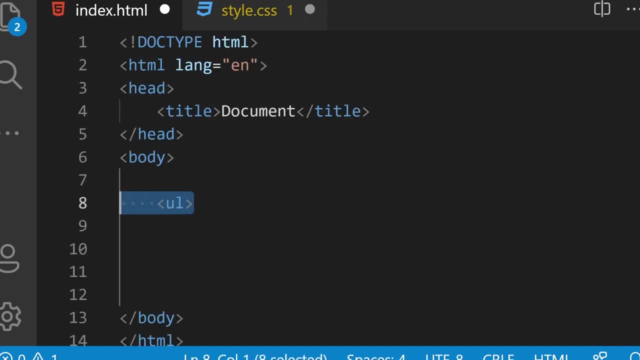 this coding from here and i'm going to also remove this ul from here as well. now let me just give example of binding. so let me just write a colon here as well. so i'm going to just mail these h1s your code, like we have first of all navigation inside this navigation, we have a ul inside this. 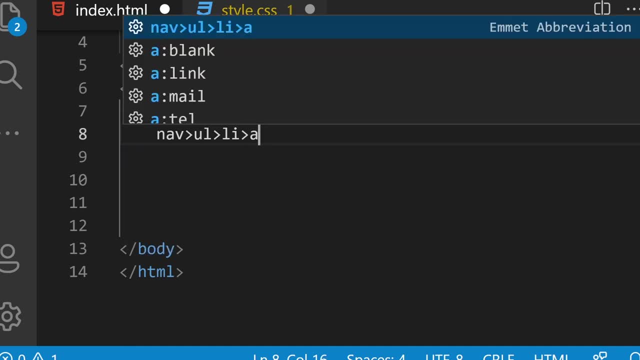 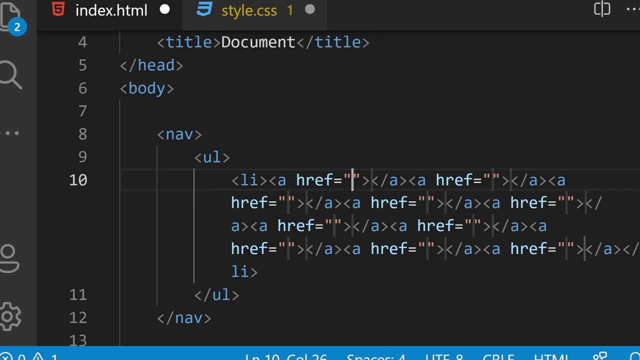 ul. we have our li inside this li, we have our anchor tag right here now. if you want to repeat like, uh, this li and this anchor tag like a lot of times. so first of all, if i just write like- let me just give example of the- if i just write like 10 right here, and if i hit tab and here you can see, 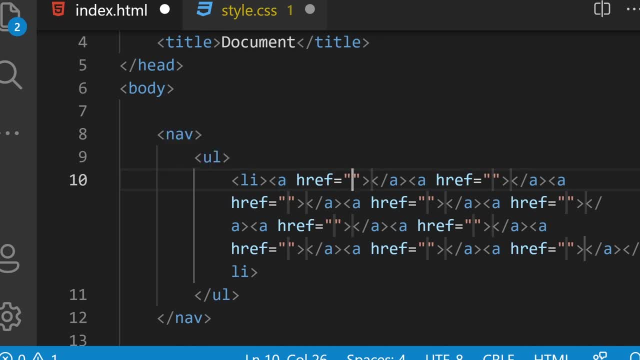 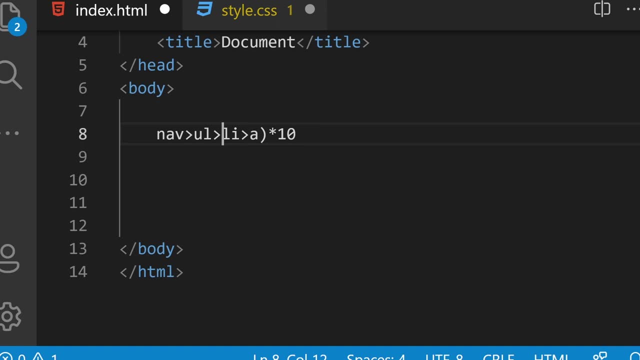 it will now gives us 10 anchor tags right here, but if you also want to repeat this, uh li with it. so you will just wrap that. first of all, you just have right opening parenthesis and then the closing parentheses. okay, so this one will be the opening parenthesis and this one will be the closing. 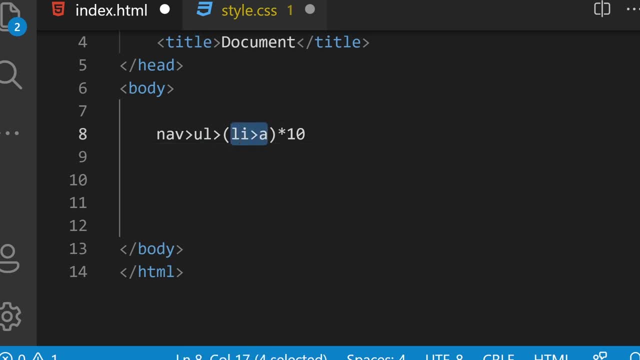 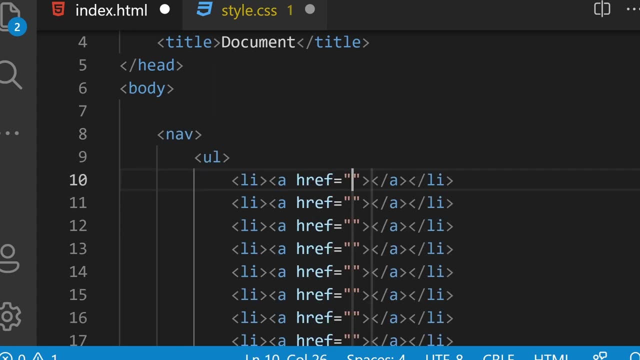 parentheses and inside these parentheses we put our elements right here. so anything we put inside there, then you can use that expression with there. so if i hit control space and if i hit enter and now here you can see, we are now getting these li's and that anchor tag like 10 times right. 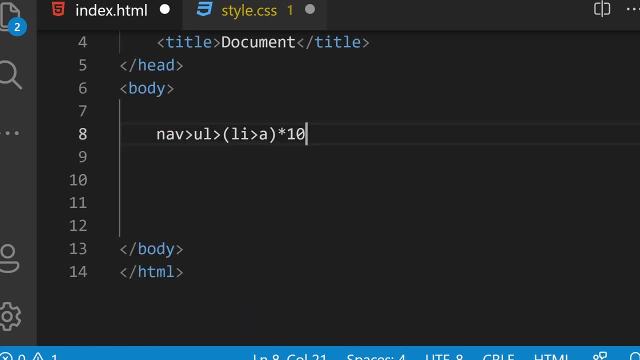 here. if i just undo it one more time, let's suppose if you also want this ul to be当 to be, print it like 10 times. so i'm going to cut that from here, i'm going to paste it right here and control space and hit enter. and now, here you can see, it will give us ulli anchor tag. ulli anchor. 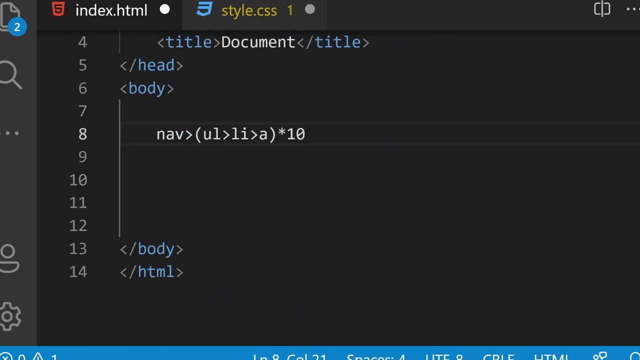 tag and so on and so forth. okay, so i'm going to remove that. so we learned about a boiler play: emits. we also learned about basic emits. we also learned about css selector emits. we also learned about nesting, multiply bindings. so now let's just learn about siblings. so sometime you would want. 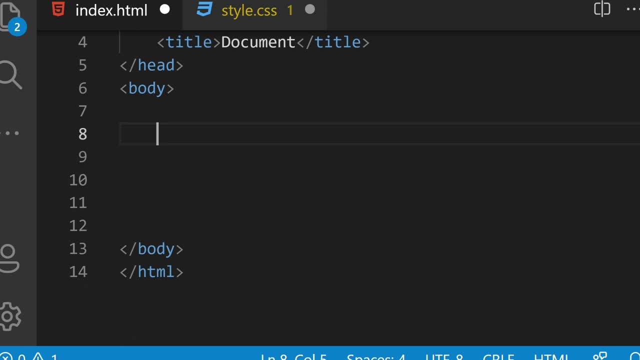 to provide a sibling inside your emirate. so how can you go about doing that? so let me just write some sort of a code. so if you want to write a sibling, so for that you're going to be using the plus symbol. okay, so you know what i'm going to just write: h1 plus h2 plus h3 plus h4 plus h5. 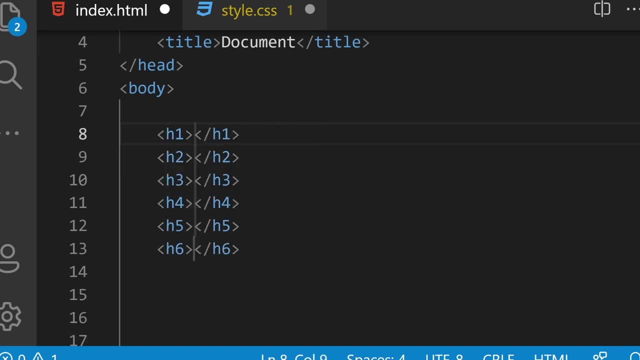 and also plus h6. and now if i hit tab, and here you can see, it will now give us h1 and h1 will have the sibling of h2, h2 will have the sibling of h3, and so on and so forth. okay, so then you can just provide, like i don't know, heading uh one and tab, heading two and tab and. 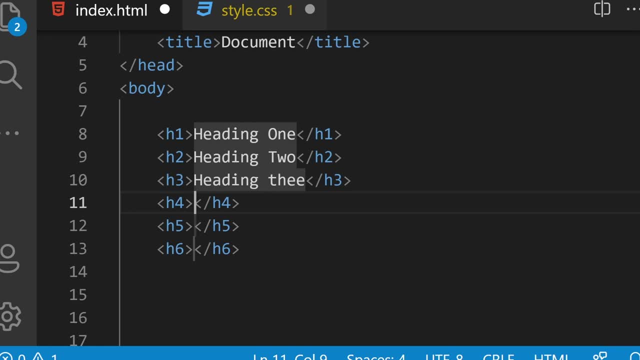 so on and so forth. okay, t heading t. i'm going to remove that from here. so now let me just write hdr like: first of all, you have a header and you want to provide a sibling of navigation to it, and then you hit enter. so here you can see, it will now give us that header and the sibling will be: 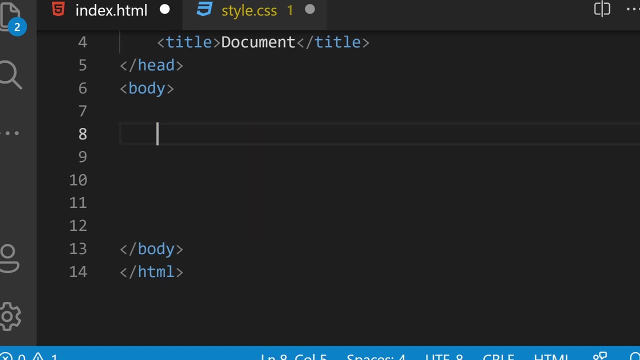 navigation right here. okay, so i'm going to remove that. and now let me just give you a real example of that. so we have a section inside that section, we have our navigation. inside the navigation, we have h1 with the class of logo and we want to provide the text to be like hello and 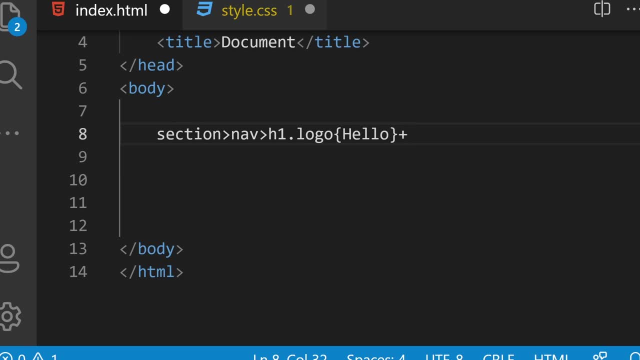 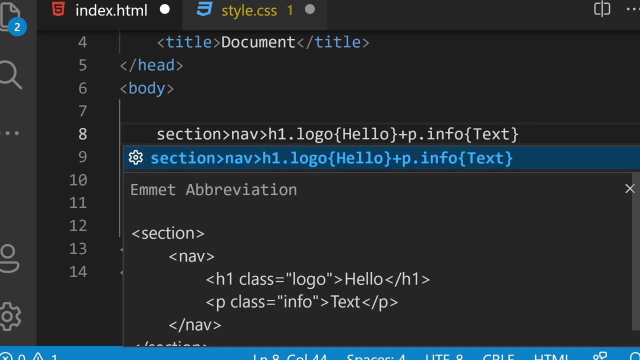 now, if you want to provide a sibling of paragraph to it so we can just write p and then with the class of info, and then we can specify our text right here and now. if i hit ctrl space and hit enter, and now here you can see, it will. first of all gives us the section inside this section we 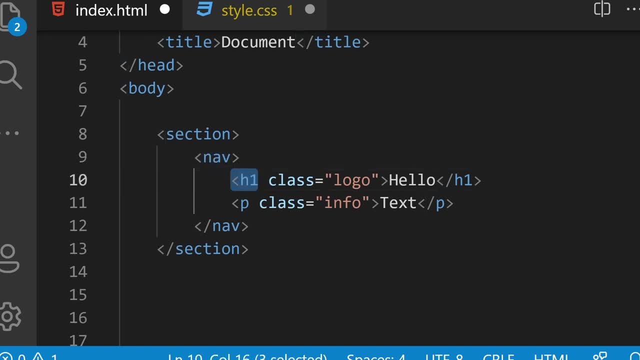 have our navigation. inside this navigation, we have h1 with the class of logo with the text of hello, and then we have our paragraph with the class of info and the text of text right here, i mean like the text of text. yeah, that's what i meant. so you can use crazy stuff like that if you want to, and i even build 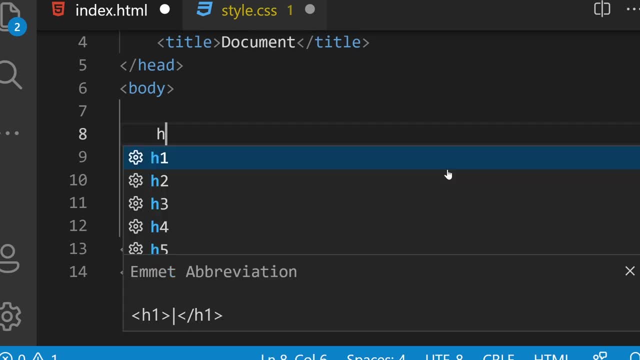 a project by just using emirates. i didn't write like, uh, h1 and h2 and so on and so forth, i just use emirates and i built a whole html and css project by using that anyways. so that was the thing. now let me just talk to you about how you can go up a level. so in some cases you want to go. 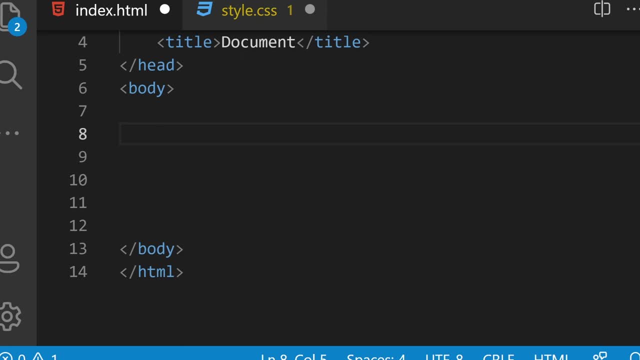 up a level in emirates. so you just have like- let me just give example- like: uh, you are now inside a header. inside that header we have our navigation. inside that navigation you would want like ul, and now you want to go up a level so you can just write a caret symbol right here. this is known as 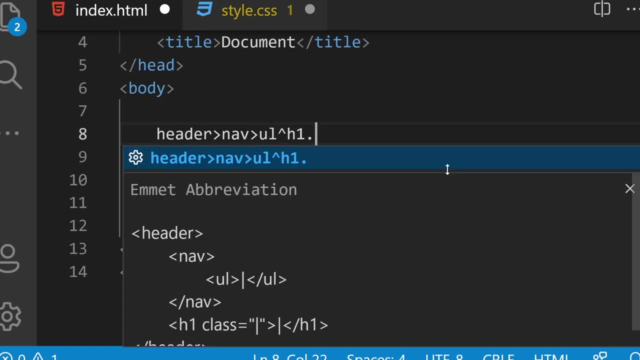 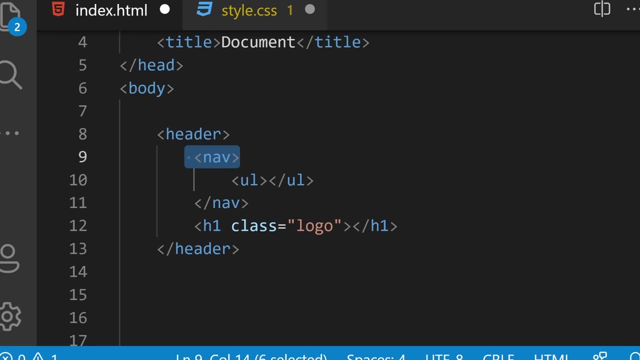 a caret symbol, and then you can just write like i don't know h1 with a class of, uh, i don't know logo. so here you can see we have header. inside this header we have our navigation, inside this navigation we have a ul, and then outside from this navigation we have this h1 with a class of logo. 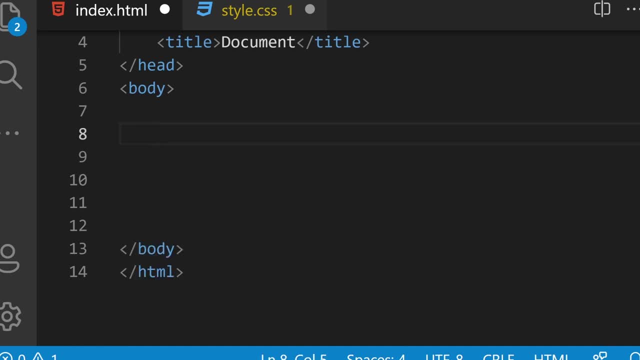 right here. so this is how you can go up a level. so now let me just give you example of that very quickly. so first of all, we will just write like hdr or header, and inside that header we want our navigation, inside the navigation, we want ul. inside that you will want our ally, inside that ally, we 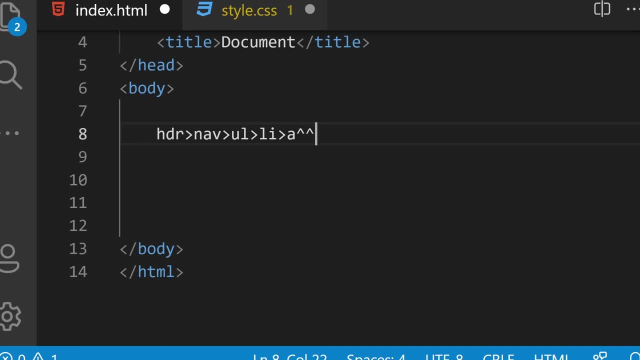 want our anchor tag and we want to go up a level and we want to write h1 with the class or not class, but with the text of text. and now if I hit control space and enter, and here you can see we have header, navigation, ul, ally, anchor tag and we 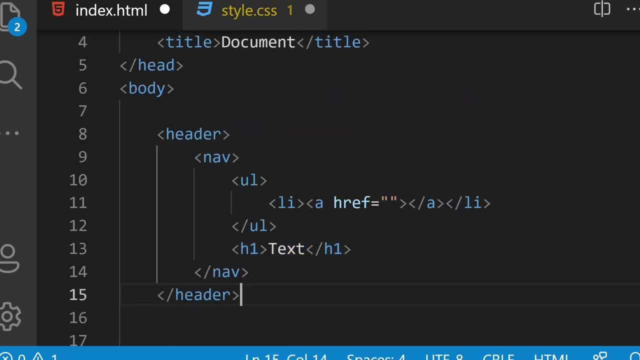 go up a level and then here you can see we have or h1 right here. I'm going to remove that really quickly, and that was it about how you can go up a level. now let me just talk to you about numbering, so we can also work with numbering in emirates. so what do I mean by numbering emirates? let me 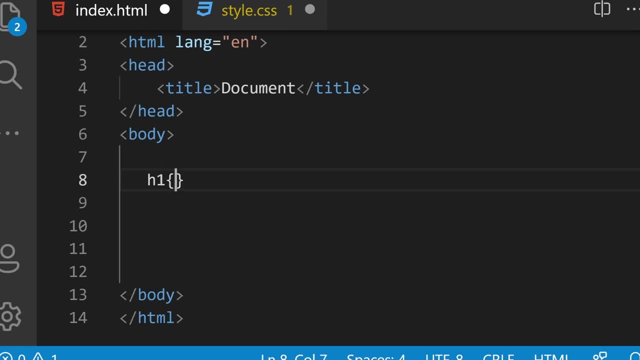 just give you example of that. so we have h1 right here and if I want to render number, so I'm going to just write a dollar sign and hit control space and enter, and here you can see we have one right here. so now, if I want to repeat it like 10 times, so I'm going to just write this: 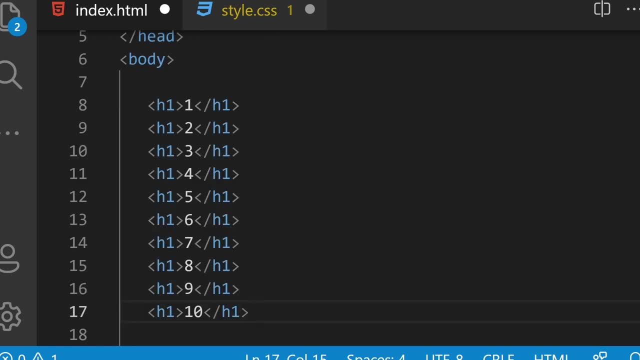 asterisk symbol and then 10, and if I hit tab and here you can see, it will now give us all of these numbers, starting from 1 through 10, right here. so these numbers can be very useful. so for that you just have to write this pound symbol and if you want to write like 00, so you can also do that. so 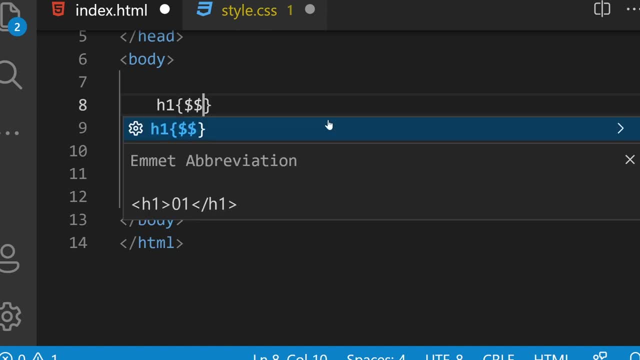 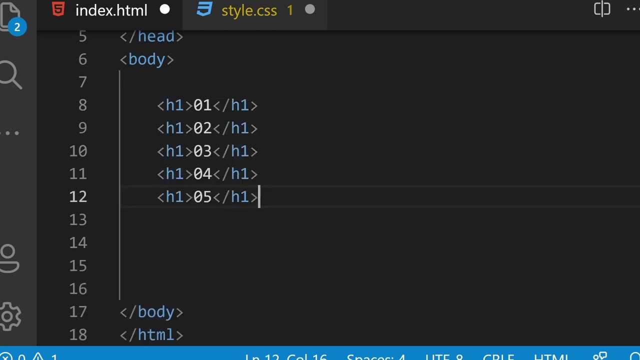 you just have to write h1 and then like a dollar sign, dollar sign. and then, let's suppose, if you want to repeat it like I don't know, uh, five times maybe, and if you hit tab, and here you can see, it will not use a 0102, and so on and so forth. 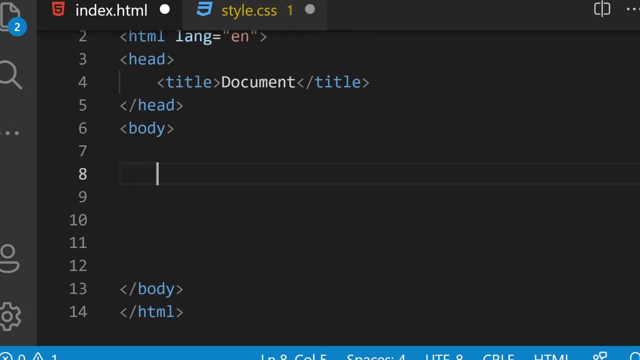 so I'm going to remove that very quickly. and now let me just show you one another example by using number. you can even use it with element names, if you want to see. we have like h1, and then I'm going to use a dollar sign and then I'm going to write my text area and I'm going to also put my dollar. 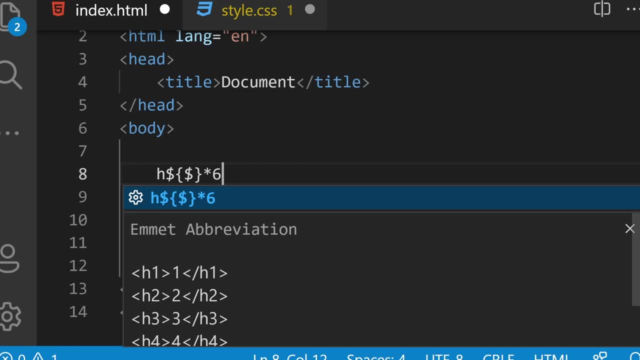 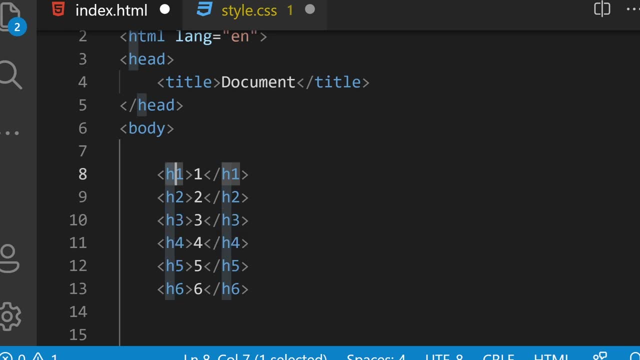 sign in it. and now let's suppose if you want them to be like six, so I'm going to just write six and hit tab, and here you can see we have h1, h2, h3, h4, h5, h6 and also the text from h1 through h6 right here. so did you feel the power of Emirates? and I know I show. 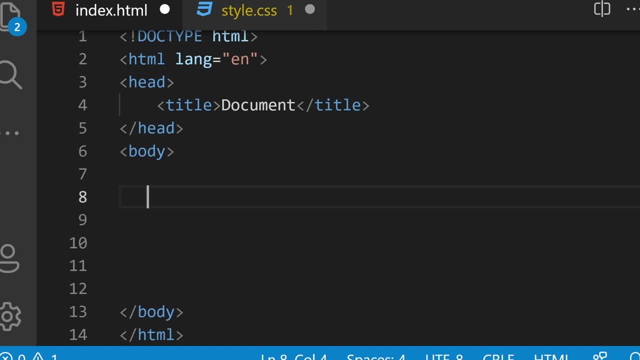 you a lot of Emirates, and you can also find a link in the description below which will bring you to my github repository, and you can also get all of their cheat sheet from there, if you want to. all right, so let me just talk to you about a very useful feature of command. 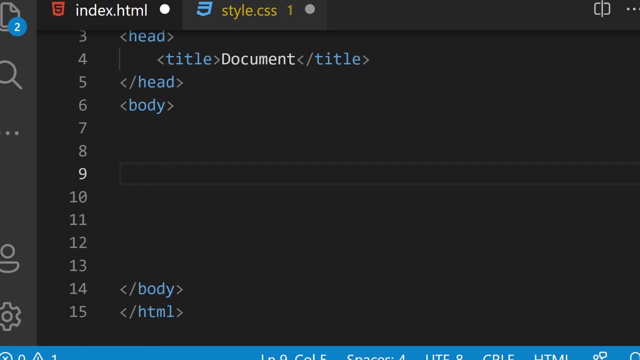 related, especially in HTML files. so let's suppose we have some sort of a header. inside that header we have a navigation and now we have a un inside there. so now, if you want to wrap this navigation in some sort of elements, so instead of doing like- uh, I don't know- writing a section and then cutting, 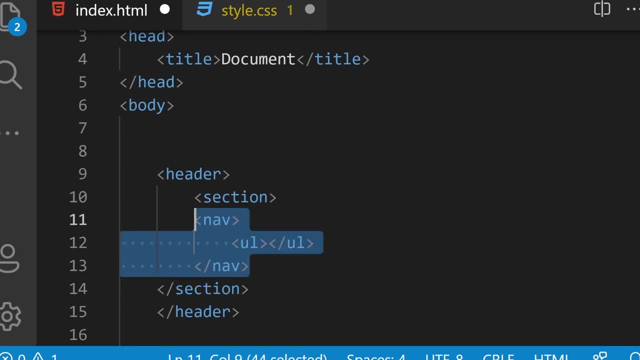 it from there and then pasting it right here and then providing your nesting in it. instead of doing all of that process, you just have to remove this section from here. remove that section and let me just undent it back. or in, okay, let me just indent it back and then I'm going to first of all, select this element and I'm going 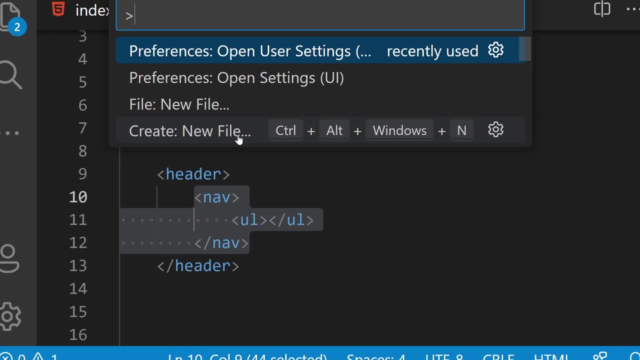 to just use F1, so it will just open our command palette right here. and what do I have to do? I'm going to just write like a wrap with abbreviation- here you can see wrap with abbreviation. so I'm going to click on that and then I have to just write some element right here. so now I'm going. 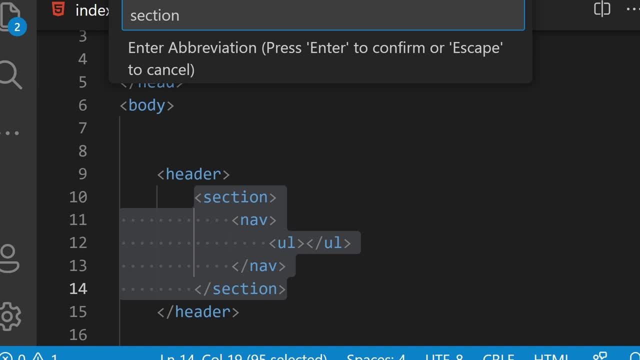 to just write section. so here you can see. it will just wrap it with section right here and I can also just provide, like I don't know, some sort of a clause to it. so the clause will be like: uh, I don't know, wrapper would be fine, and now if I hit enter. so here you. 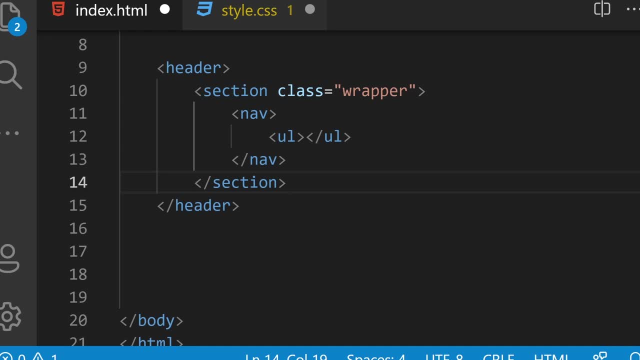 can see. it will just do it like that. it will just do it very, very quickly. so that was just a very handy feature of uh- what do we call it? command palette inside HTML files. so I'm going to remove that and let's just write H1. let me just write H1 of hello, and then we have some sort of an uh span. 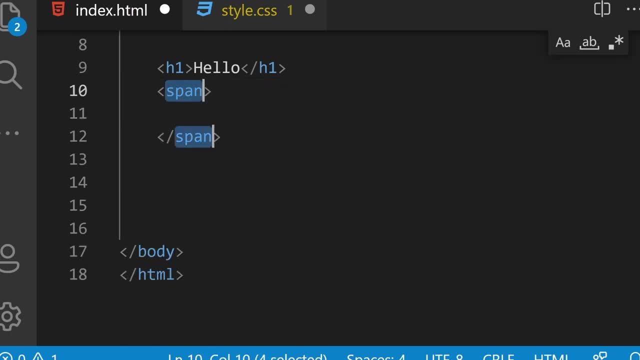 and yeah, inside this know what, let me just write section, and let me just write article inside that section, article this one. and now inside this article we would have a section, inside this section you would have, or a side. and now let's suppose, if you want to wrap this aside with something else, so you can just 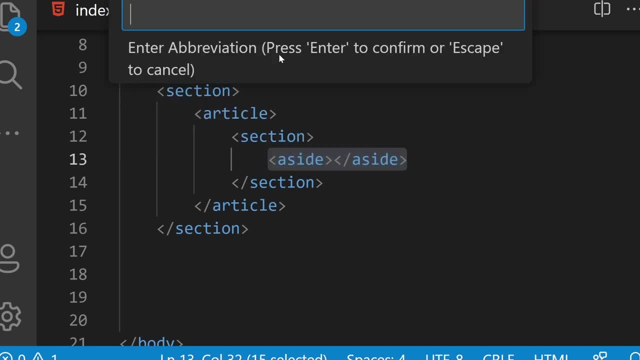 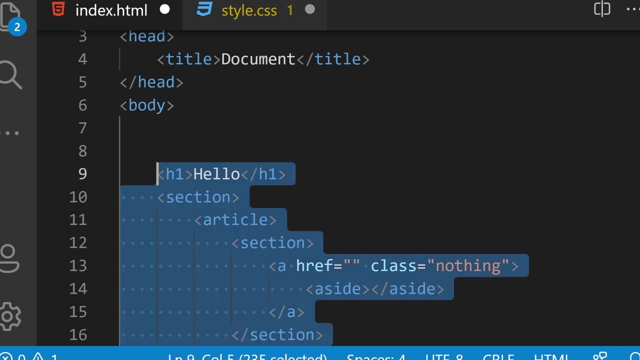 hit f11 and we can just write a wrap it with abbreviation and then we can just write like anything we want. so we can just wrap it with anchor tag with the class of nothing. okay, and now if i hit enter, so here you can see, it will just wrap it with this anchor tag and these things. 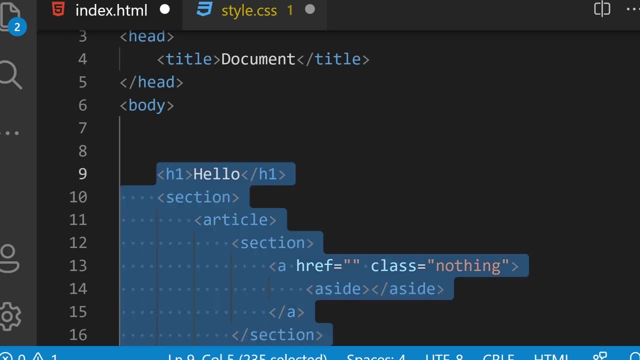 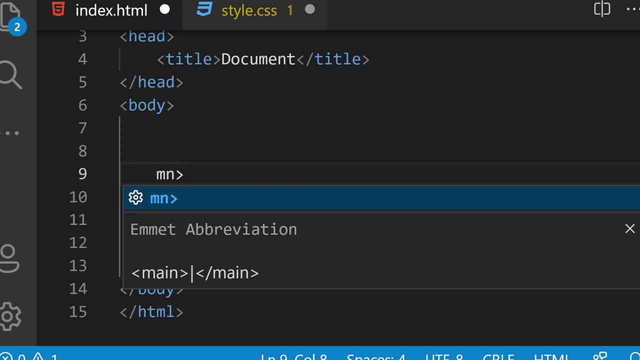 are very, very useful in html files. so now let me just put all of that together in one image. so let me just write mn for the main. then inside that man, i want to write a section. inside that section, i want to write article. inside that article, i want to write header inside that header. 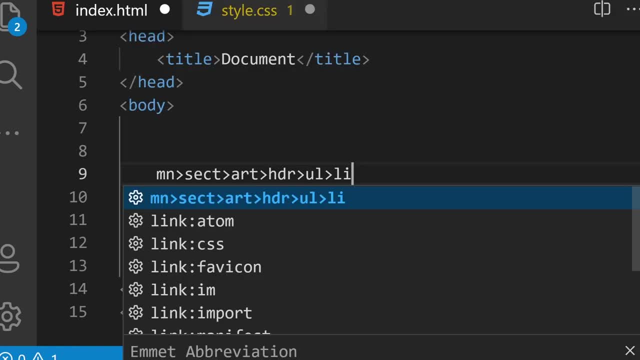 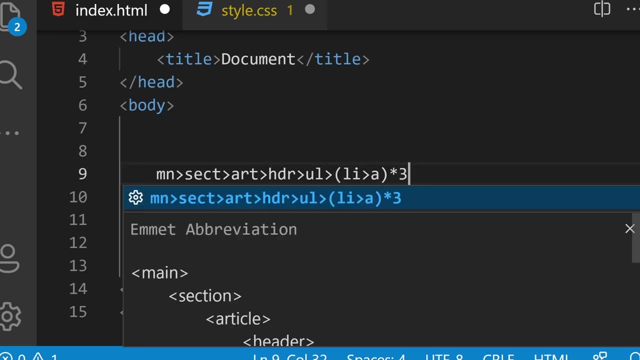 i want my ul. inside that ul i want my li and inside that li i want anchor tag and i want them to be, i don't know, maybe three times. so i want to just repeat it three times. and then i want to go outside. so i'm going to just write a carrot symbol to go outside from there and then i'm going to. 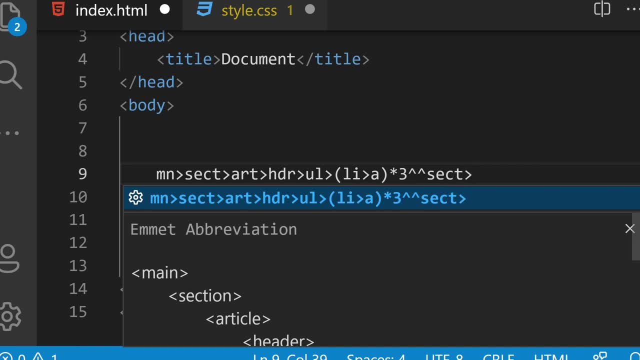 just write a section one more time and inside this section we will have our h1 and i'm going to just write a text of like welcome in it, and then plus and then p for the paragraph, and then i'm going to just put my lorem in it. okay, so if i hit control space and enter, and now here you can. 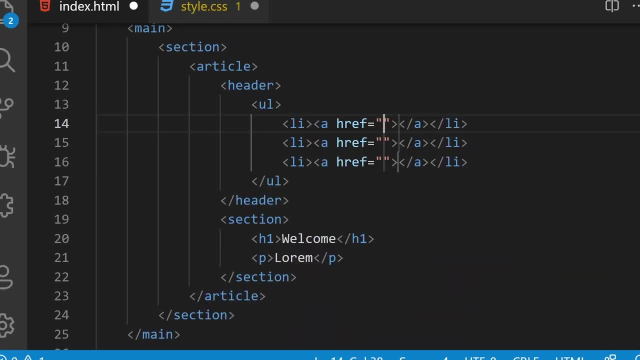 see we have. first of all. let me just zoom out. first of all we have our main. inside that man we have word section, then article header, ul, ally, and then we have our section, and then we have h1 with the text of welcome and then, underneath this h1, we have our paragraph with the class not a. 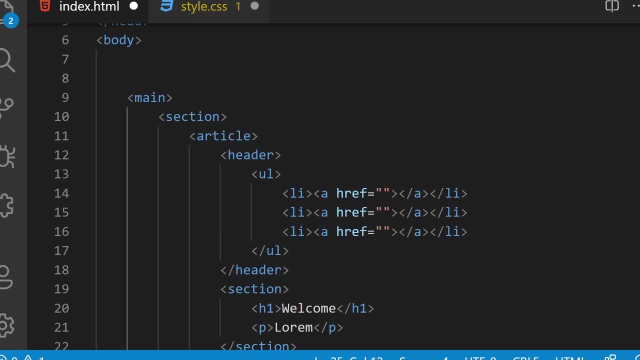 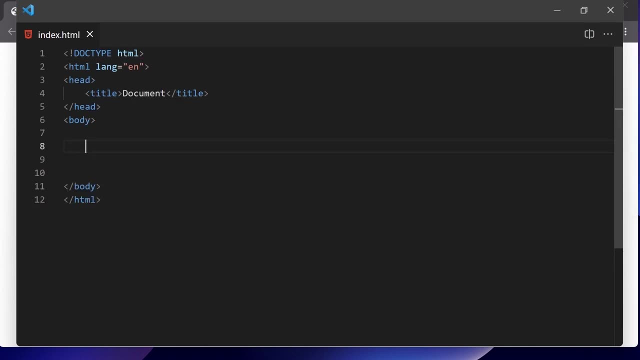 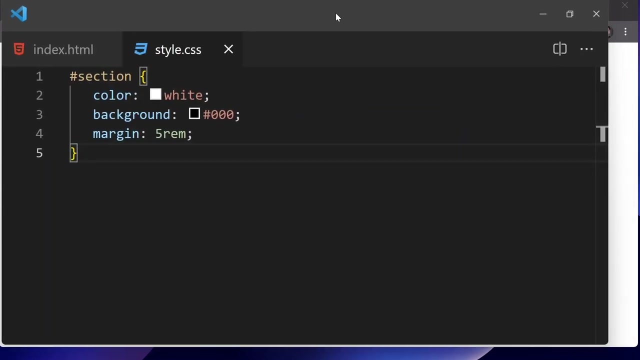 class, but with the text of lorem right here. so this is how you can use emits inside your projects. and, by the way way, i forgot to show you the css image. i already showed you the html emits, but i forgot to show you the css image. i am very sorry about that. so in css we don't have built-in image so we can write. 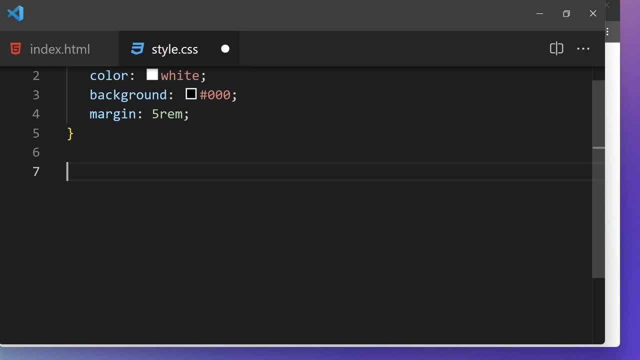 our code a little bit faster, but we don't have a built-in- uh, what do we call it? image? so i'm going to remove this coding from here and let me just write some sort of a selector right here. and then let's suppose, if you want to provide a padding, so you just have to write p and hit tab, and here you. 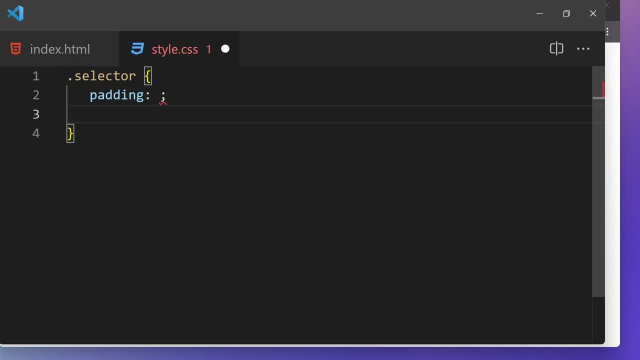 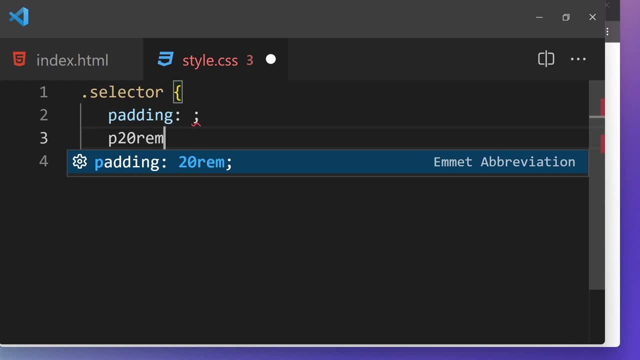 can see, it will just auto complete it for you. and let's suppose, if you want to provide some sort of a value inside that padding, so you just write a p and like 10 or 20 and you can also specify the room, what do we call it? the unit, if you want to, and here you can see, it will just provide that. 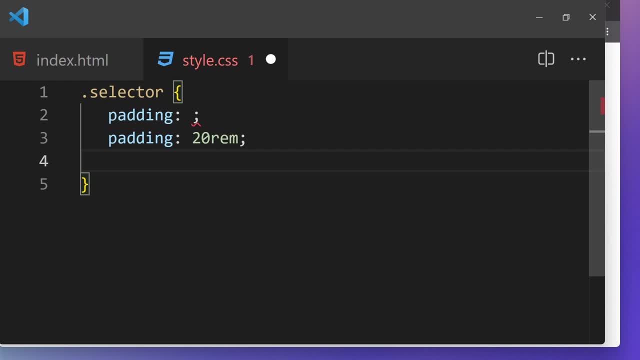 unit. if you want to get a margin, so you just have to write the first letter of anything you want to write. so i'm going to just write like margin, like m, and if i hit tab and here you can see, it will just auto complete it for me and also. 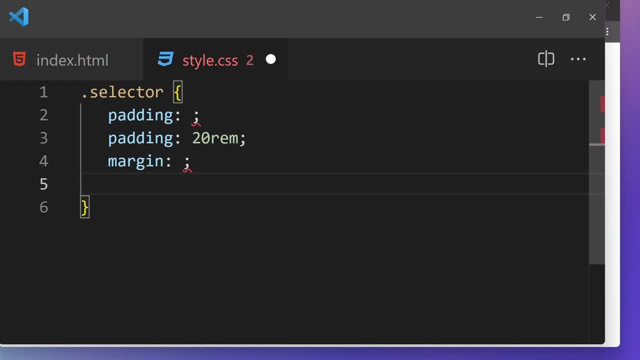 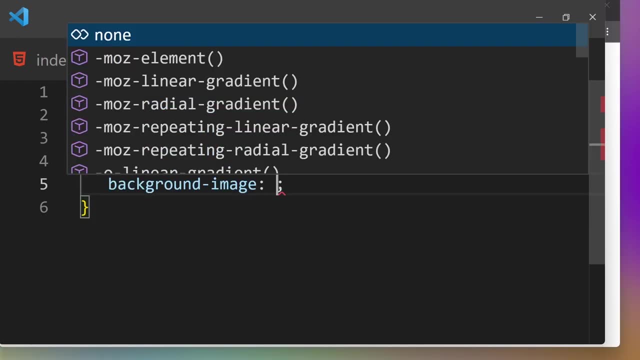 know if i want to get a background color or background image, rather. so i'm going to just write b, g for background, and then i am g, and if i hit tab and here you can see it from now just auto completed right here and we can also just write a color. so i'm going to just write bgc and 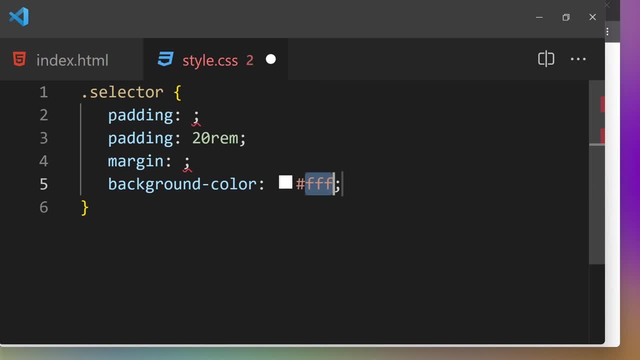 if i hit tab it will just auto complete it for me and it will even give me that totally white color. so if you want to get a text colored so we can just write c and hit tab and here you can see it will now give us that color and it will just fill it with this. 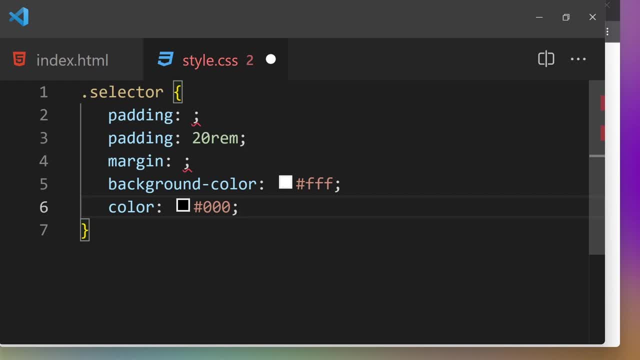 totally black color. okay, so if you've watched my uh html css course, so you already know these stuff. but if you don't, in case, so here i'm showing you right here. so if you want to just write like uh, i don't know, uh, display of flex, so you just write df and hit tab. it will give you display. 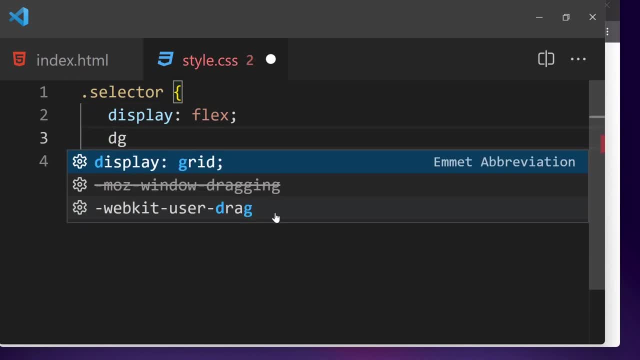 of flex. if you want to get a display of grid, so you just write dg and hit tab, it will just write display grid for you. if you want to try display block, so you just write db. and if you want to get like display in line, so you just write di and for this display in line. so nothing special. 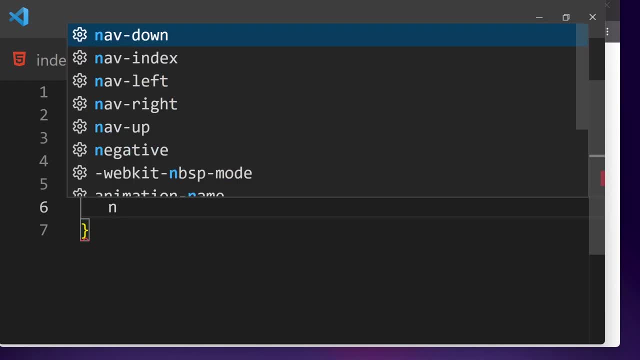 so if you want to get something, so you just write the first layer of it and hit tab and it will just auto complete it for you. okay, so like colored so c, hit tab. background color so bgc, hit tab and boom. this is how the css emits work. 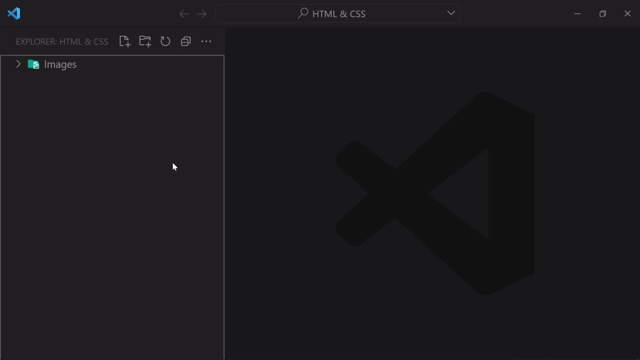 all right guys. so welcome to your first project. attention, this video. you will find a link to my github repository and if you want to follow along with this project so you can use these images, or you can use your own images if you want to. so i just kind of want to mention that in the first place. so what do you have to do? we are 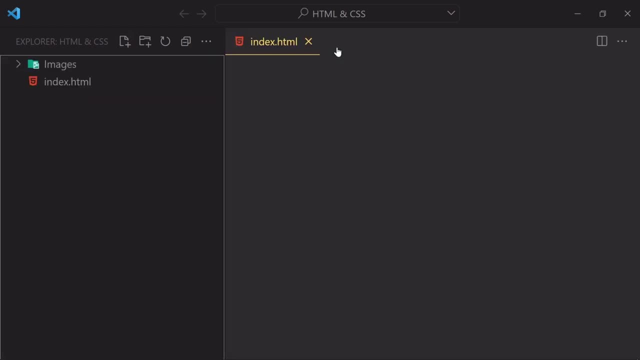 going to start working on our first file. so i'm going to just create a first file, indexhtml. now let's just create a new one, which is stylecss. and now let me just make that a bit bigger and hide that upper bar. and now we are totally good to go. so what do we have to do? first of all, we are. 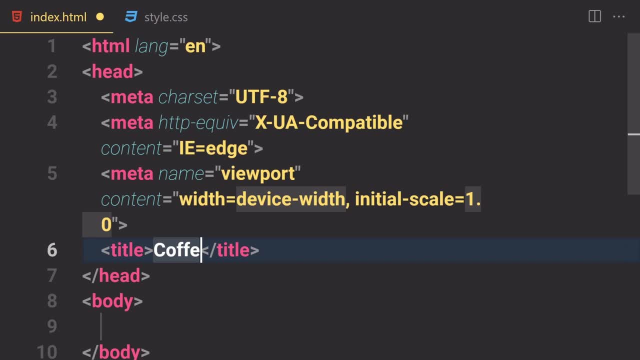 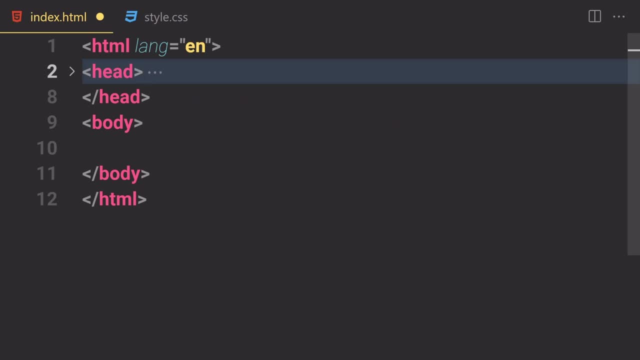 going to create our first file, indexhtml, and i'm going to change this to like a title. to be like a coffee, let's just link it with our css file and i'm going to just hide this metadata from there and save our file, right click on it and open it with a live server, so we can now open our project. 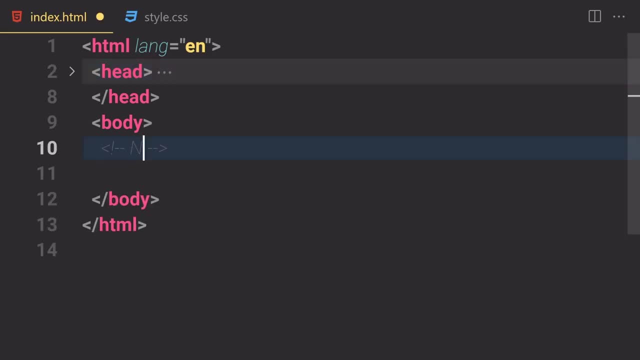 in a live server, all right. so now let's just start working on our navigation. so i'm going to write a nav in here, i'm going to write a nav opening and closing tag and then i'm going to write like h1 off with the class of logo and i'm going to just put a logo in there. 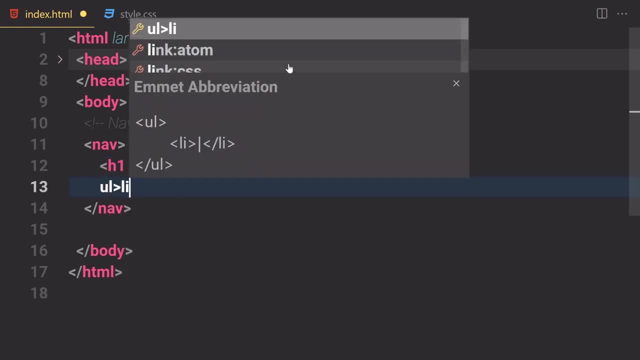 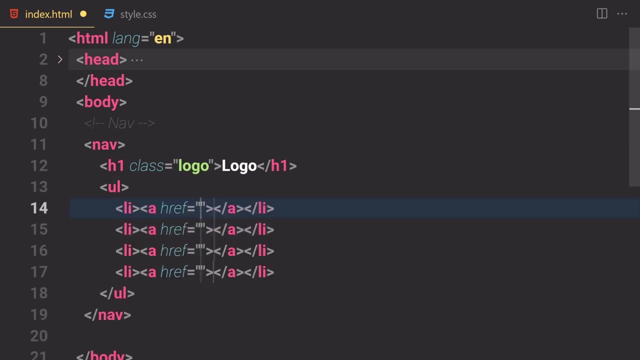 i'm going to zoom out a bit and here i'm going to write like a ul, then li and then anchor tag, and i'm going to just uh write like i don't know, maybe four of them. i want to just put a four in there. it will not go to anywhere, so you just write like a home then about. then it will go to the menu and 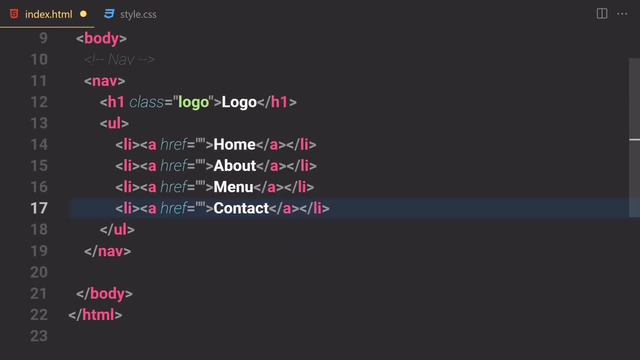 then, finally, we have our context section right here. okay, so now, if you sell a file- and i know currently things totally awful, so now let's get into our css file and now let's just start working on it. and let's get started. so what we do? first of all, we would need a font to grab from a google. 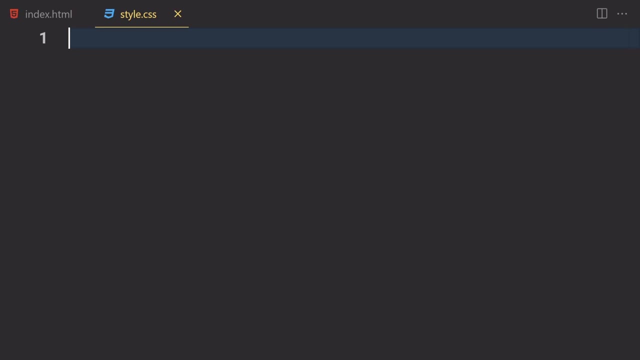 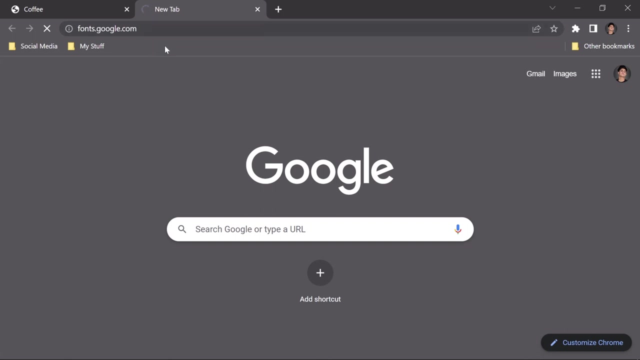 font. so we are going to be using a font, card, play, fire or paper, whatever you want to call it. so to grab that, first of all we have to go to our font start googlecom. so if you go to this font start googlecom then we can search for that font. okay, so my internet connection is totally awful in. 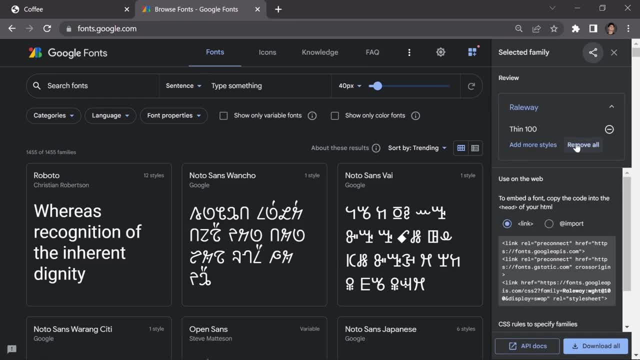 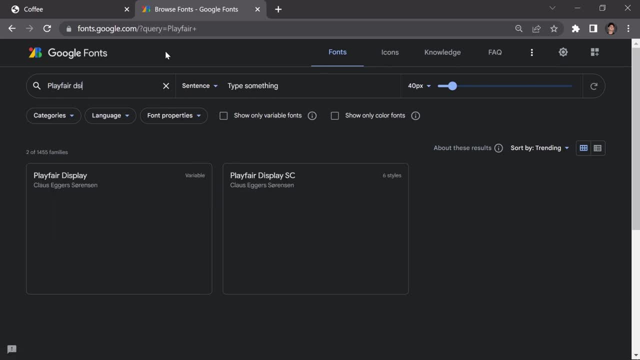 this video. okay, we have to wait for that. so what i'm going to do, i'm going to just remove all of these styling which i have for my previous project and i'm going to just type like a fire and display: so okay. so i just have to write a d in there and i'm going to choose this one. 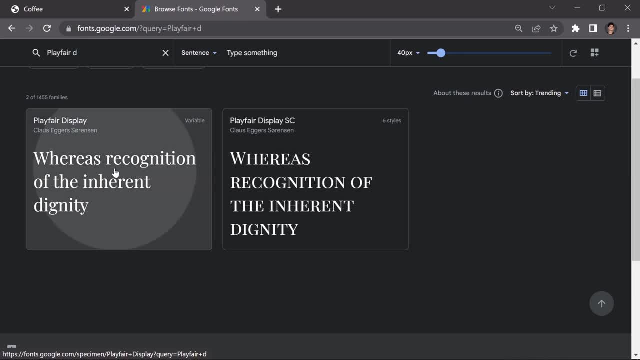 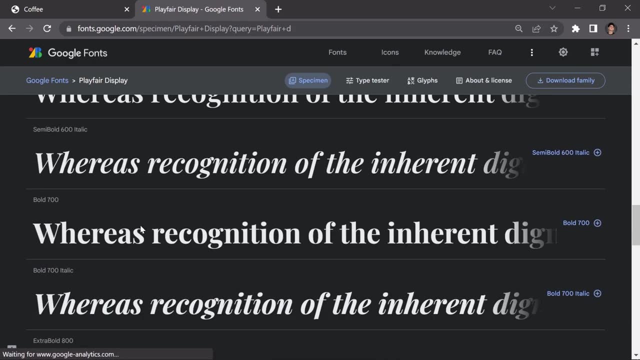 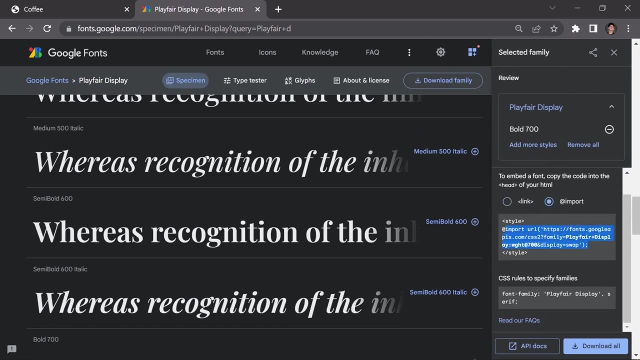 because i guess we use this font. uh yeah, i'm going to just click on the first one. the other one is awful and now let's just select word 700 width right here. so i'm going to just click on this 700 width plus, then click on that, click on this import. you already learned all of that stuff. 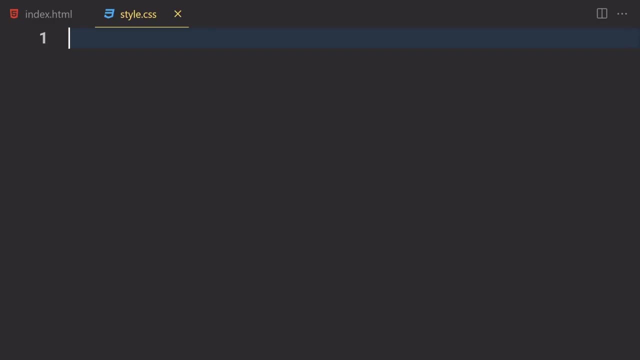 i don't have to revise myself, but i'm speaking, i don't know why and what for, because i have already teach you everything which you need to know to build this project. but anyways, i'm going to be talking and you have to listen to me, or, if you don't want to listen to me, so click on that. 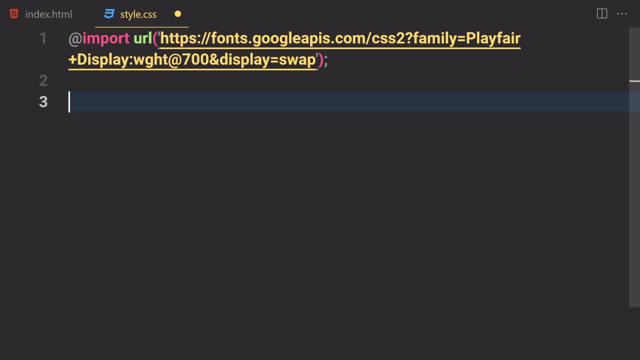 mute button and you can listen to your favorite music while writing your code anyways. so what do you have to do? first of all, let's just create a few variables. i'm going to just create a variable for our main color, and the main color we are going to be using is d, e, a, b, five f. 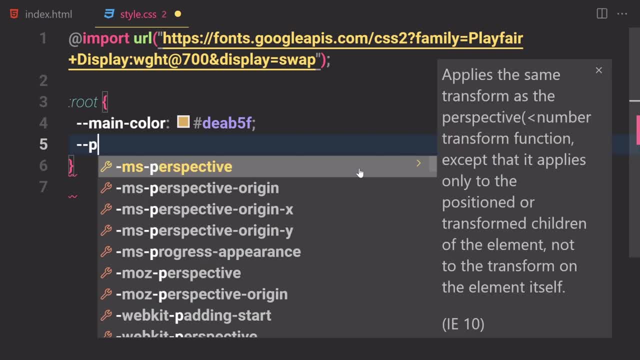 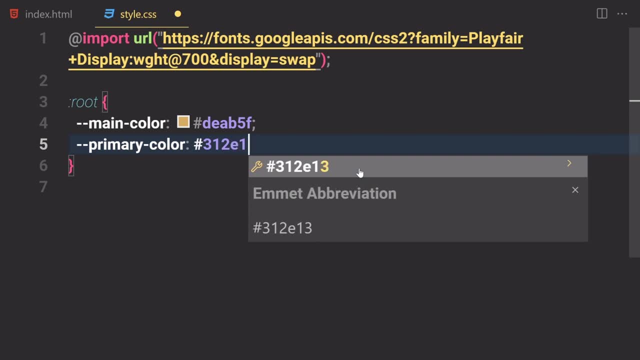 so i'm going to just create a variable for our main color and the main color we are going to. so this is going to be our main color for this project. and now the primary color we are going to be using is that uh, three or one, two e, two e. so this is going to be our primary color for this. 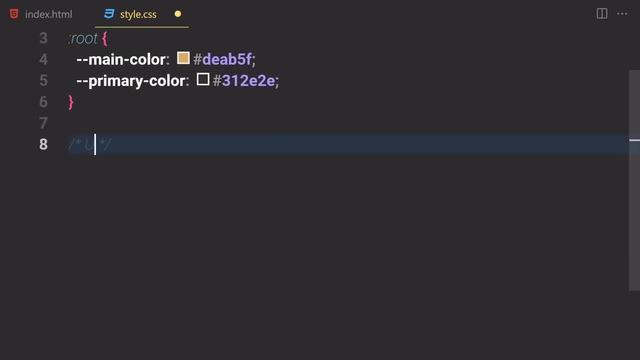 project. so if you sell that now, let's just also write our utility- uh u t i l i t y classes as well, or styles to be precise. i'm going to just write a buttons. i'm going to just write a class for a button, first of all, and now let's just provide a padding of 10 pixel to that button. 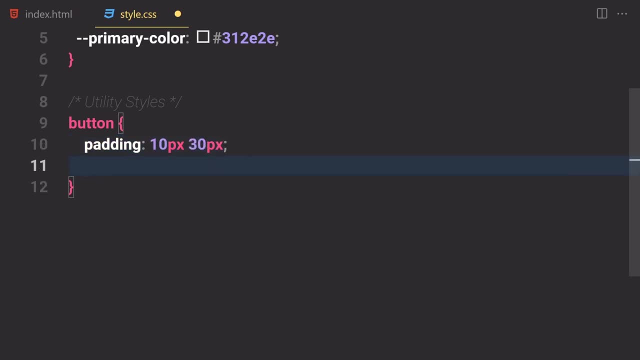 and also the 30 pixel bottom, like 10 pixel will be for the top and bottom and 30 pixel will be for left and right, and we are going to be using a background color of that main color which we just declare. and now let's just remove that border from all of these buttons and the cursor will be. 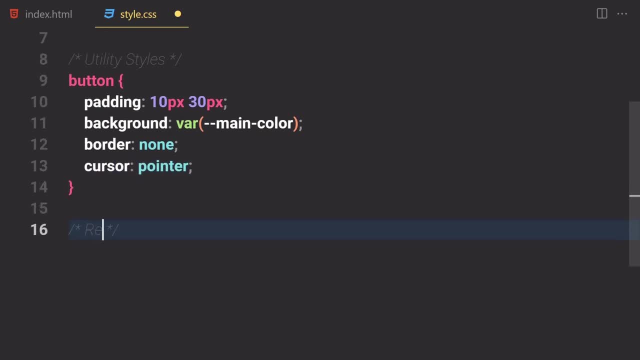 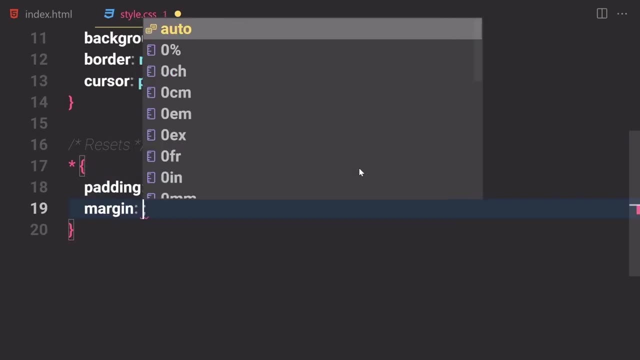 by default pointer, all right, so now let's just write a reset. uh, for ourselves. if you want to write a reset, so it's not a crazy resets- we just have to write a padding of zero, margin of zero and box sizing will be totally border box. all right, so now let's just write a reset for ourselves. 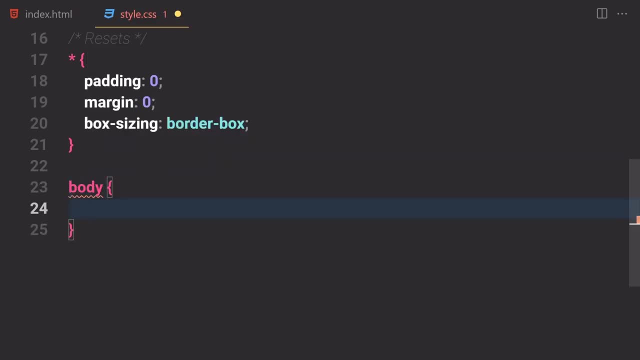 now let's just get in to our body. so what do we have to do? i'm going to just um change the background color to be like i don't know. i'm gonna write 100 e and then 0 f. it's not of, it's zero. so 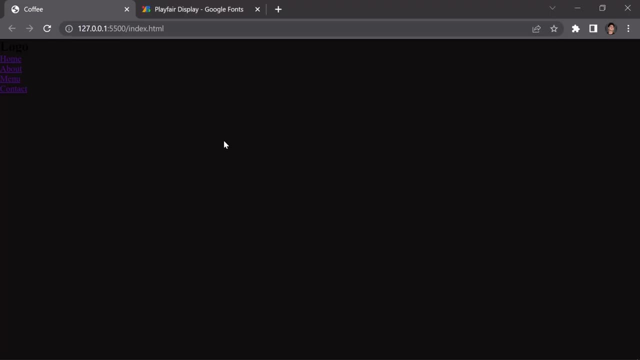 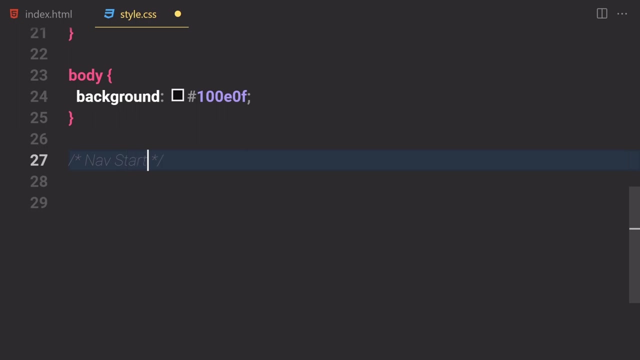 if you save a file, and this is how currently things looks like. all right, so now let's just work on our navigation. so i'm gonna write a navigation start in here, navigation start. and now let's just start working on our navigation. so i'm gonna just select my navigation first of. 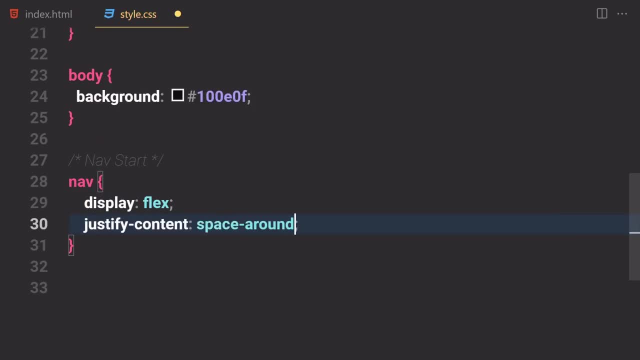 all and left click with that, and so obviously we're going to have a時候. it probably will write signals. actually, let me click on our navigation sign. refrigeration on, of course, little fax in here and thenay. we're going to need a display of flex in it. justify corner will be spaced around. 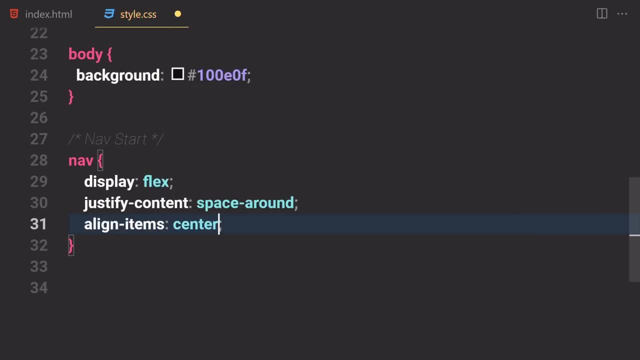 because we want these items to be like all around each other. we don't want any spaces and stuff. so i guess we do want spaces. that's why we just write space around there. so now we are going to be using aligned items of holy center and now let's just write a color to be totally pure white font family. 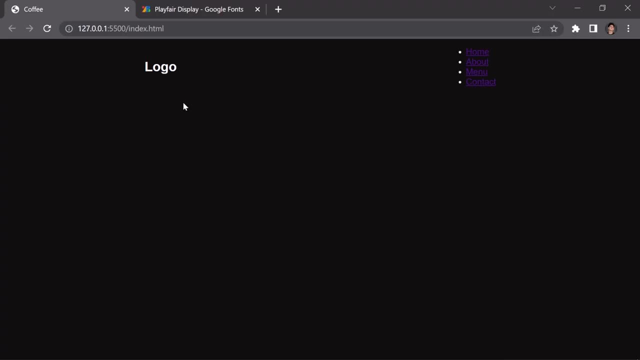 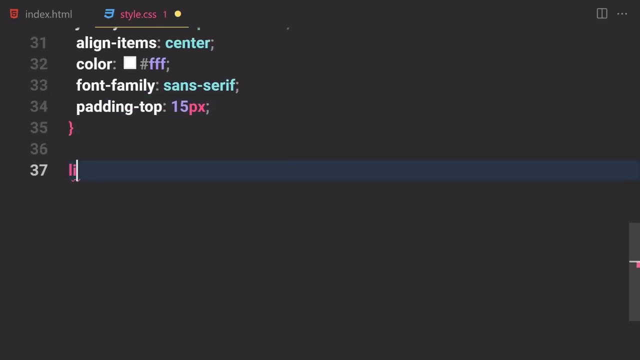 padding top will be 15 pixels. so now, if you save that. so now, this is how currently things looks like. now, let's just select this li right now and provide a display of inline turd. so i'm going to select that um li right now and i'm going to just provide a display of inline turd. so now let's just 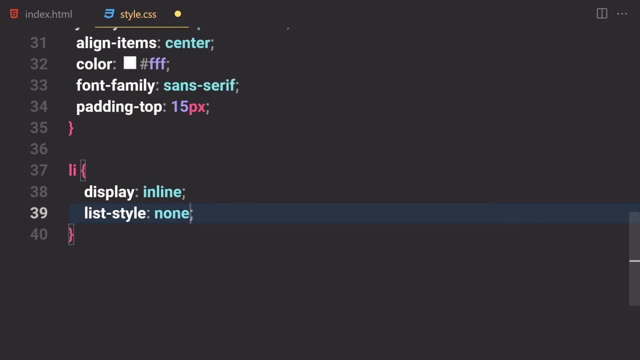 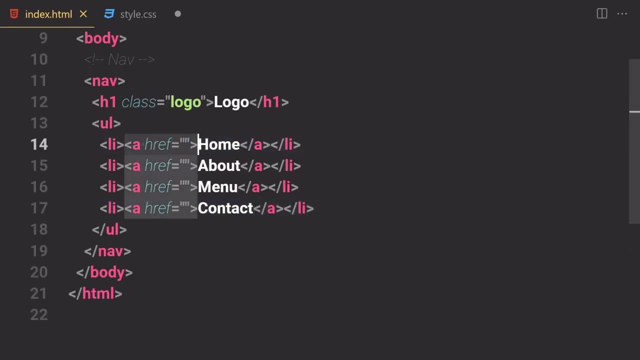 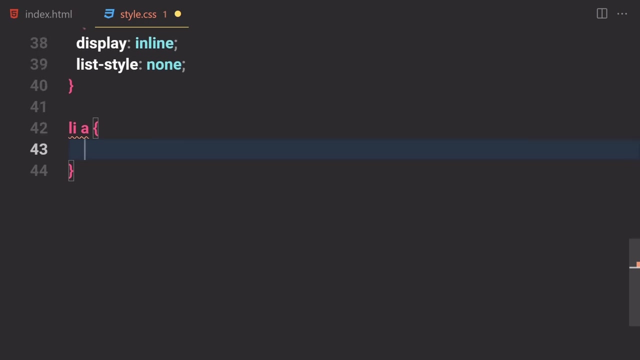 remove that ugly list style of none. so if you save a file and boom, this is how currently things looks like. and now let's just select our anchor tag, which is these anchor tags? okay, so now let's just select that real quick. uh, i'm going to write like li and then a. we want to select all of the anchor. 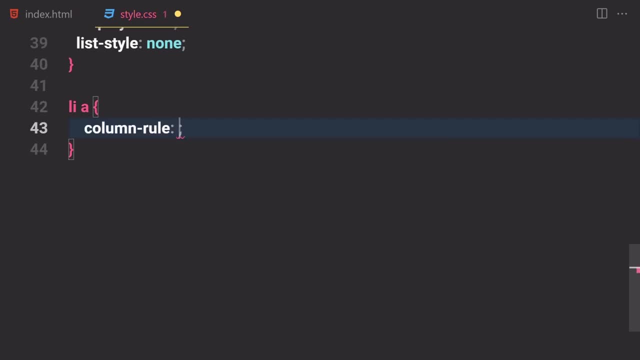 tags, which is inside the li, and we want to change the color of them to be like: um, let's just change the color to be like totally white color, and i'm going to also provide text decoration of none, because we also want to remove this ugly line right there. so i'm going to make that to 100. 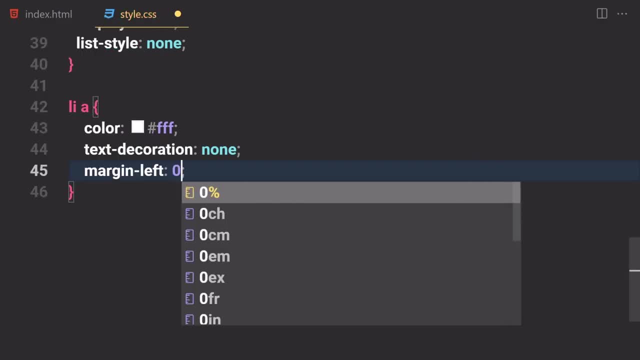 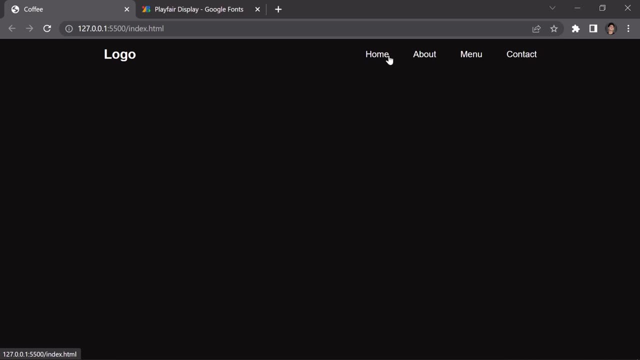 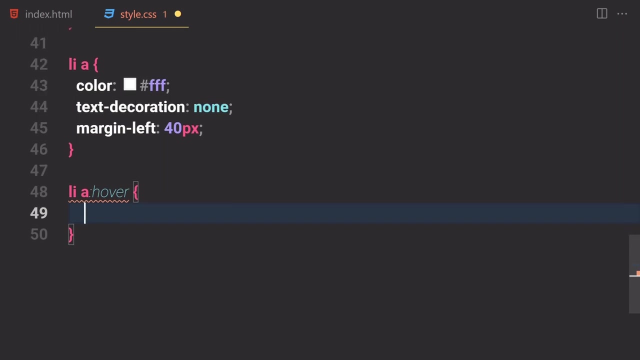 and margin to the left will be like 40 pixels. so now, if you save that- and this is how currently things looks like, so you know what- i forgot to include that hover effects. now let's just also provide that hover effect on it. so if you hover over to our anchor tags. so what do we have to do? we just have to provide a border bottom. 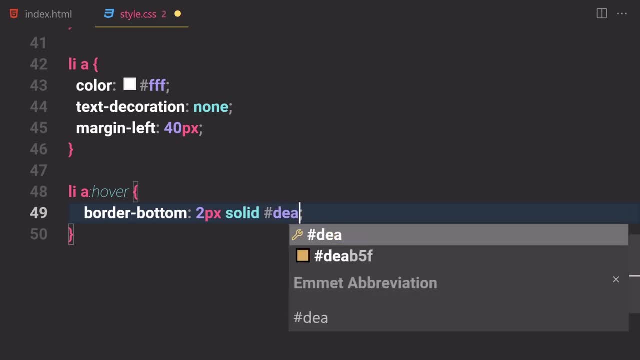 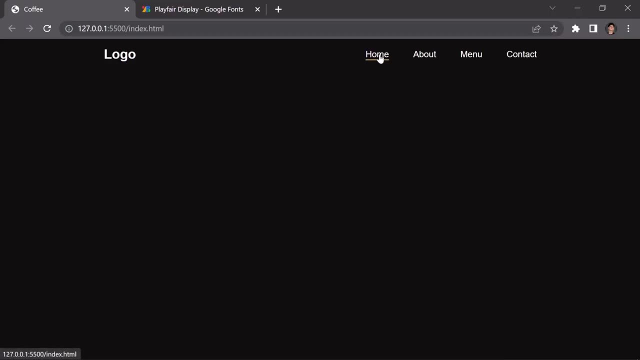 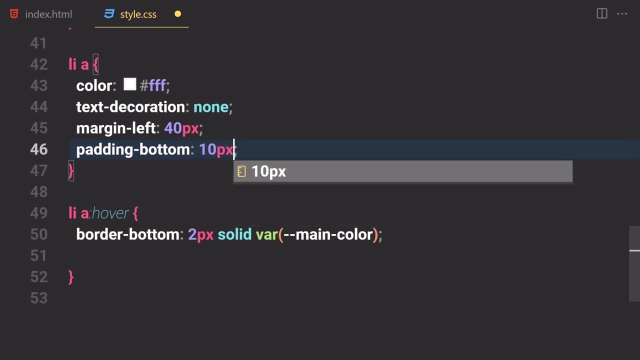 of two pixels, solid, of that kind of a, dea, b, five, uh, you know, we can use that primary color, uh, so if you save that and now if you have our mouse overturned, this is how currently things looks like, but we can also go a little bit better, so i'm going to write like border bottom of like 10 pixel. 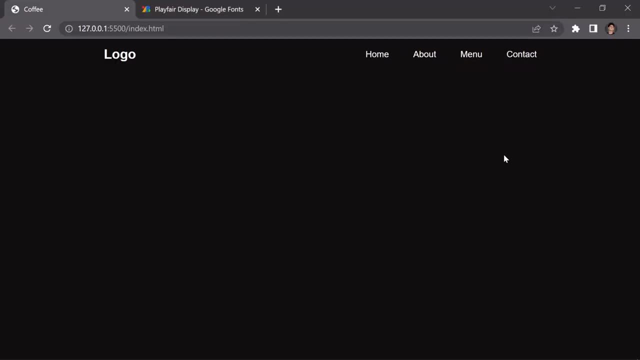 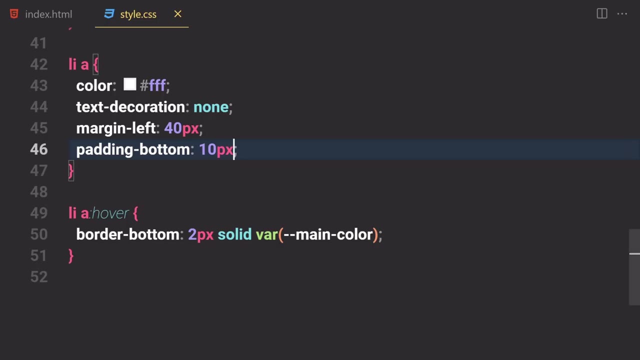 and now, if you have a mouse and turn your mouse on to the other side, uh, just a little bit better have ordered. so this is how currently things looks like if you make it smaller, like so. so it's totally responsive. by the way, by not using- uh, what do we call it a? media queries. so now we 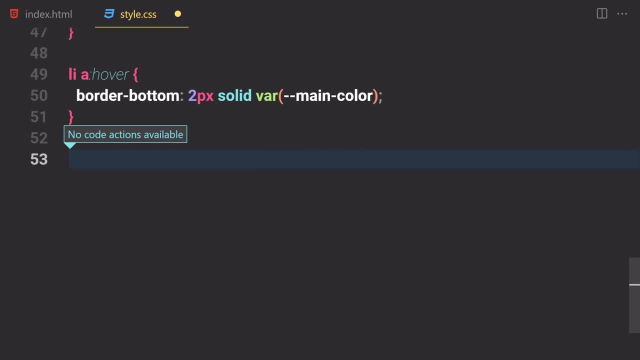 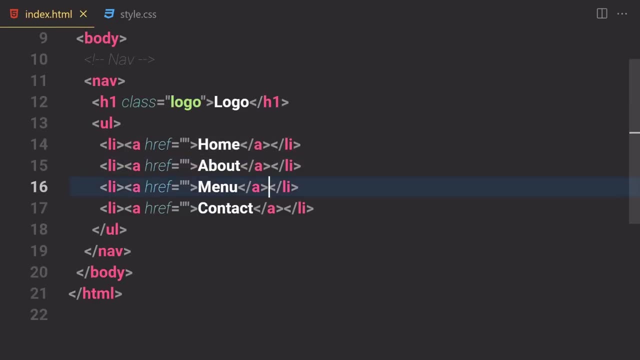 are totally done with our navigation, so i'm gonna just write a comment for myself. okay, i can't get my comments. uh, nav end. so this is the end for our navigation. so now let's just start working on the header area. so if you want to start working on our hair area, so for that we just have to write. 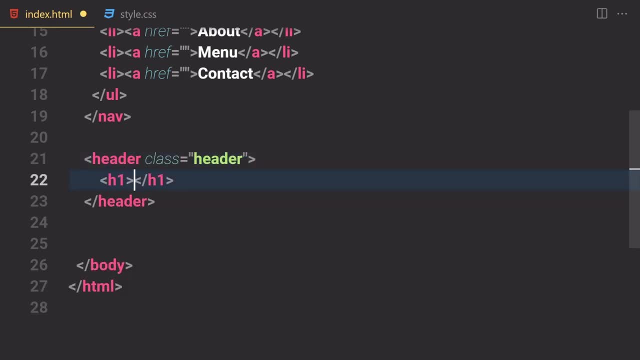 a header with a class of also header, and inside this hair we are going to be using h1 with a class of main headings. okay, so i'm going to just write like a start your day. now let's just select our h1 off with the class of primary heading and now let's just write with or coffee. so now let's just. 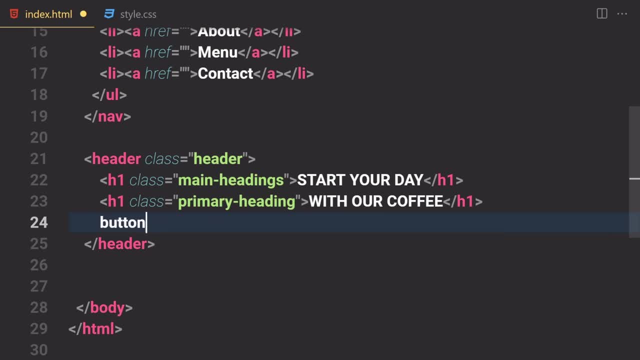 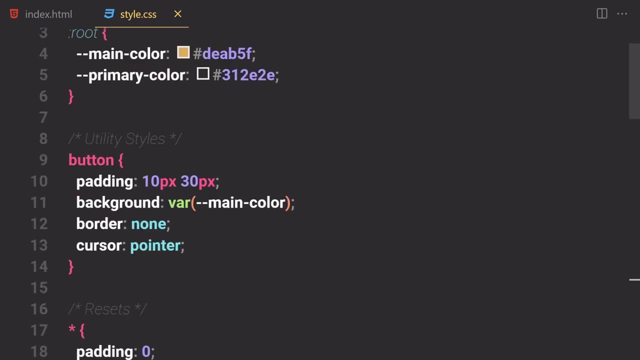 create our button right here and with the class of- oh my goodness, bt rub ton with a class of main btn. let's just write like shop now and now. if you save that, the button will have these classes. that's because we write these classes inside or utility classes right here, but the other content will not. 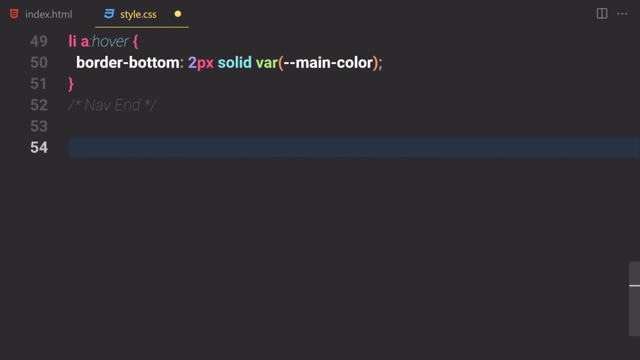 be styled by default, because we don't write any styling for that. so now let's just provide a styling for our header area. so we are going to be writing our header- start in this case. so what do we have to do? first of all, we just got to select our header first of all, which is the header with. 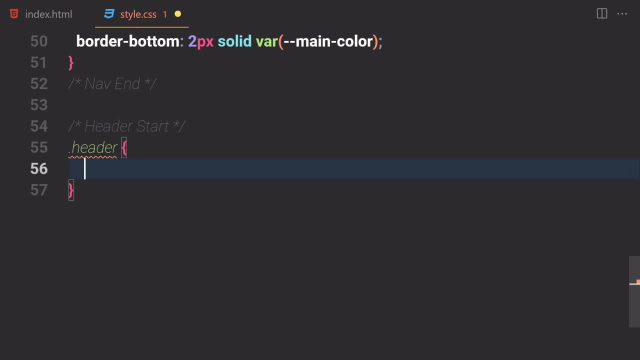 a class of header as well, so we are now selecting that by using our classes. so now, what do we have to do? first of all, we want to attach some sort of a background to it, so i'm going to remove that real quick and let's just write our url, select our images- and i guess the image was um this one. 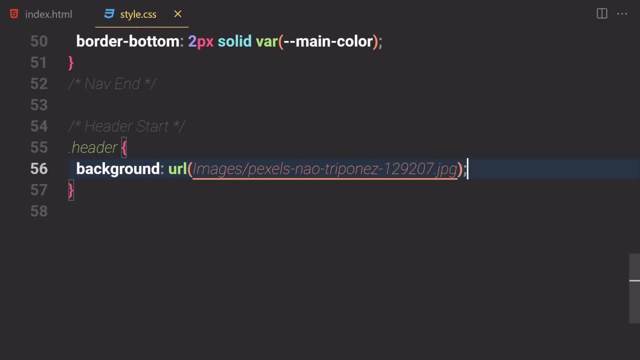 the last one, i guess. so if you save that- and yeah, we cannot see this now- let's just make our positioning to the center. so i'm going to just write a background position of holy center and i want to also provide a background size to be covered totally, and i'm going to also provide a height of 100 vh to it, and what do we have to do? 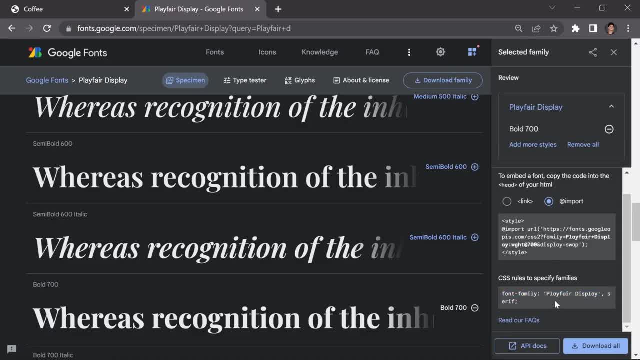 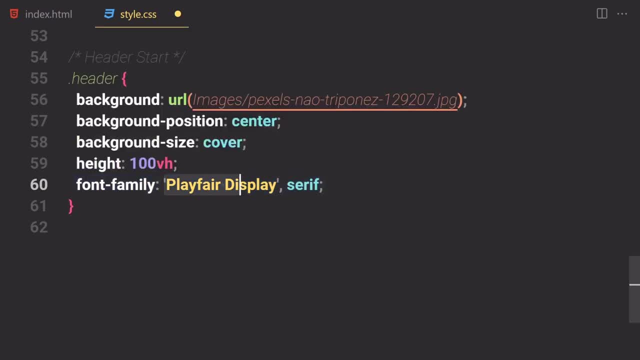 we are going to be using that font, which we grab real quick, so i'm going to just copy this font family from there and copy that and paste it. so if that font is available, use this font. if that font is not available, then use this serif one. so if you save them and now here you can see this- 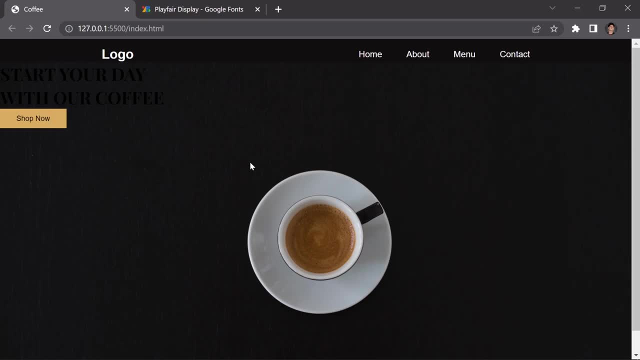 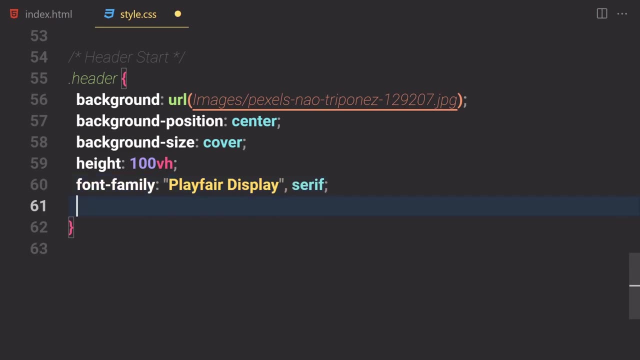 not only at the center, right here and now. let's just use our font. we already use a font family on there, but it's not looking that much also, so for that we have to center that and stuff. so we are going to be using a font where of totally. 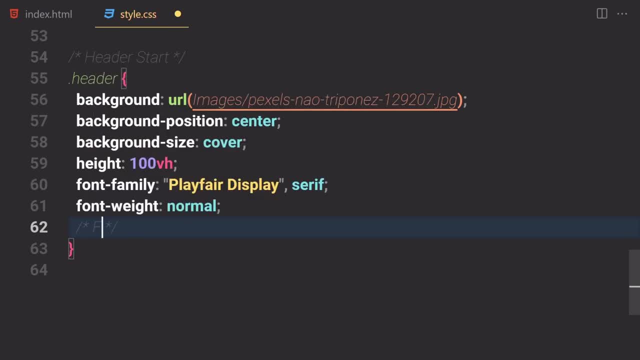 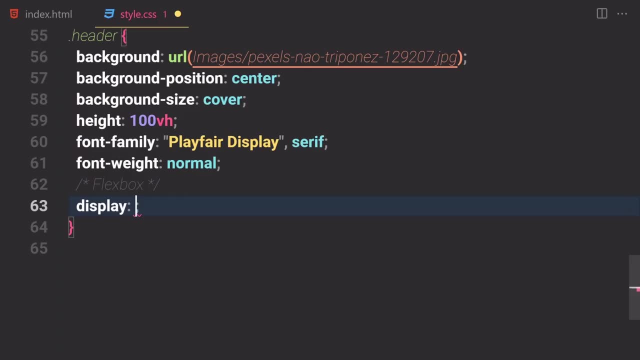 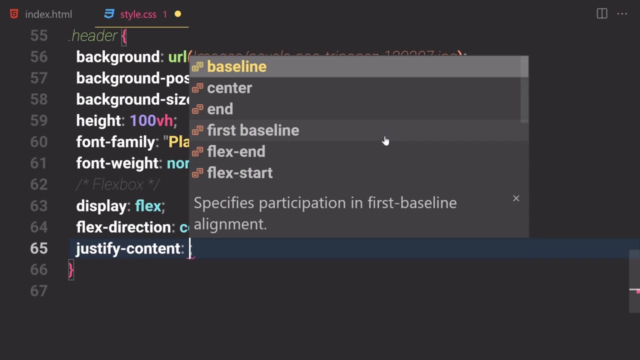 normal and let's just write: or uh, flex box in here let's just do our flex box magic. so if you want to make that like totally at the center, so for that we can use display of flex. and now let's just use a flex direction to be totally calm. and now let's just write a justify content to be 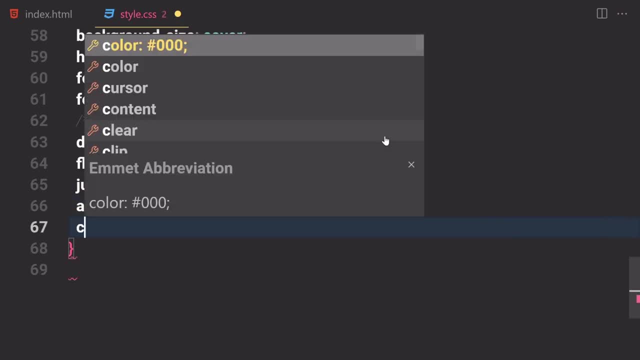 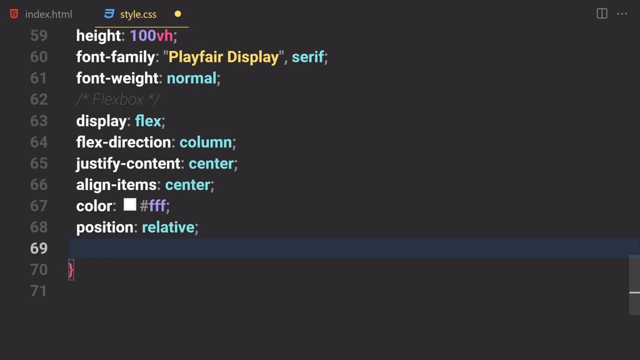 totally at the center. align items will be also center. and now let's just write a color to be totally white and let's just write a position of relative to it. we are not going to be worrying about responsiveness just right now, but we will take care of that once we jump into the end of this project. so if you save, 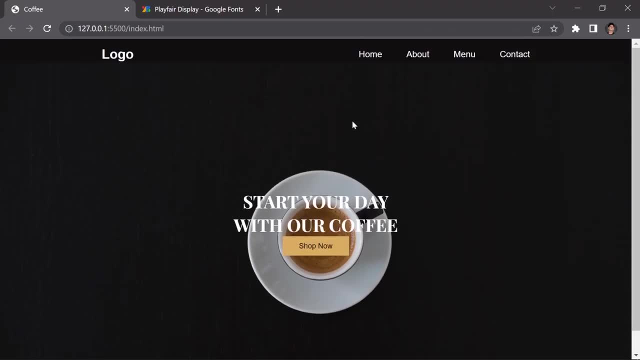 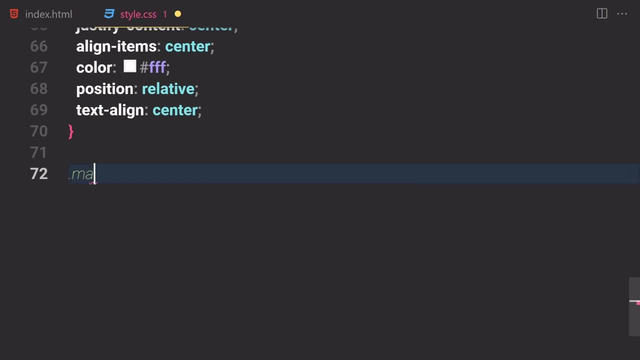 that and now currently things looks like these: i know you're so full, so now let's just start working on our main headings right here, like this one: so now let's just select their main headings right now. so this one is a position relative right here. i'm going to set that to at the end. so you guys. 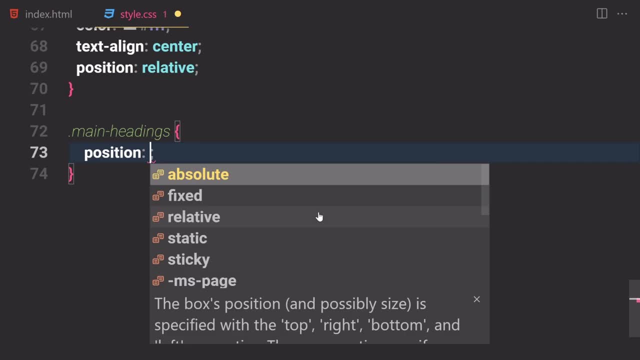 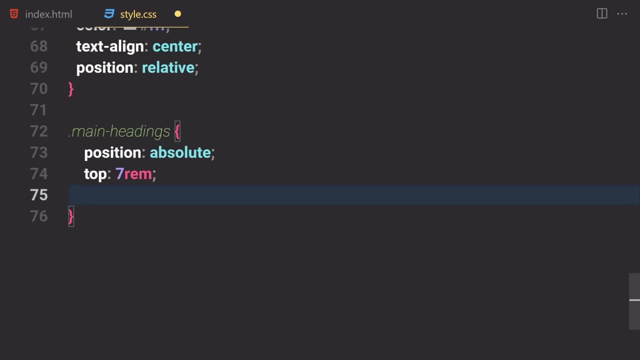 can see everything if you're reading this code, and now let's just provide a position relative to it. so i'm going to create a position on absolute on there, and now let's just use a top will be like sound rim. i know for a fact that it will be required like a sound rim, and now let's just use. 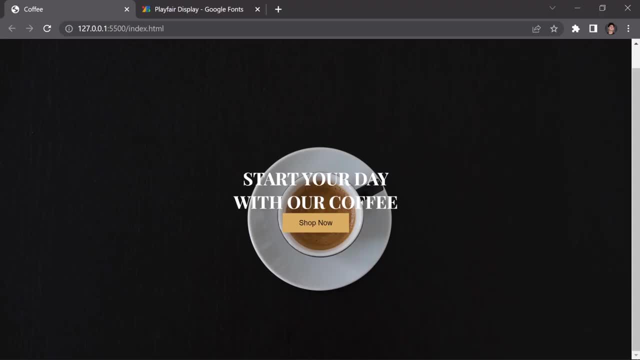 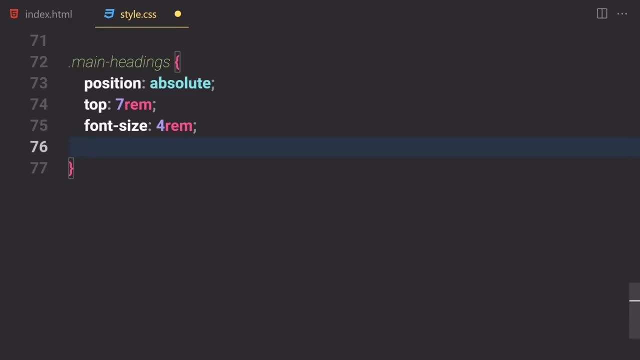 like font size of forum and if you want to work with this image, so you just have to figure out like how much of uh positioning i would need. so in my case, i just provide off sound rim of positioning. and now let's just also do- what do we call it, that word spacing. i'm going to provide. 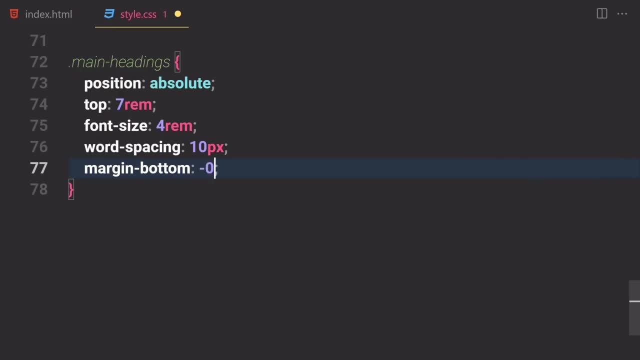 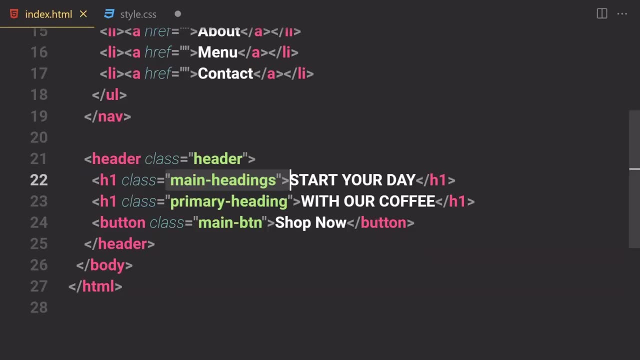 10 pixel of world spacing in each, and i'm going to provide a margin bottom of minus 40 pixels. so if see, if you saw that, and this is how the first one looked like. all right, so now let's just work on. or primary headings. so that was for the main headings, now let's just work on, or 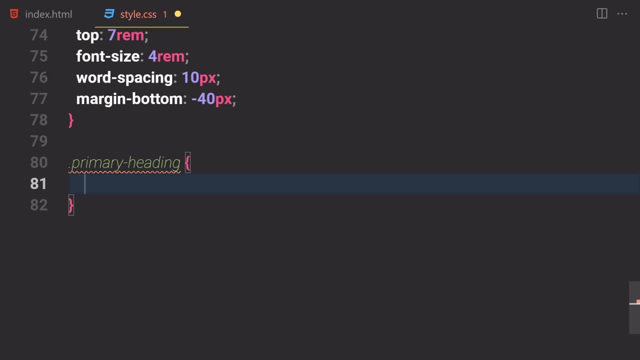 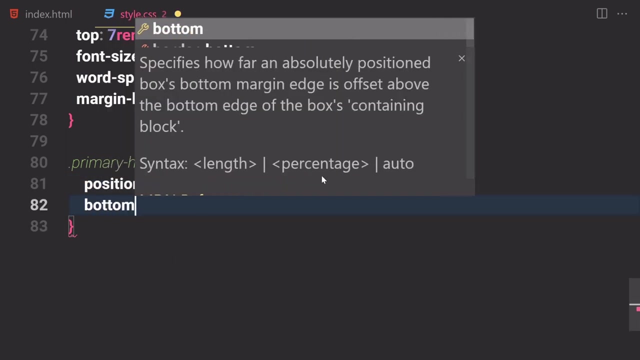 primary headings. so, uh, okay, so it's heading or headings. it's singular, it's not plural. okay, i can't pronounce that plural anyways. so now let's just write a position, position of absolute, right here and now. let's just provide a bottom of forum of positioning. 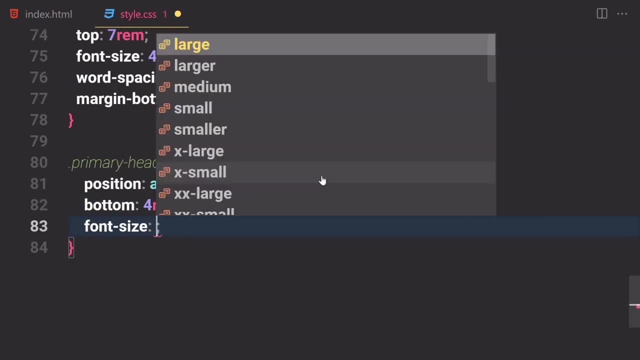 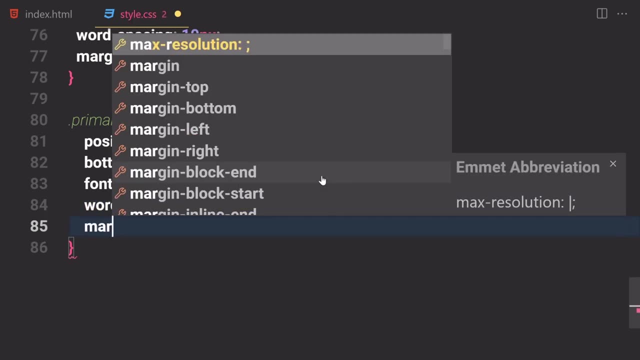 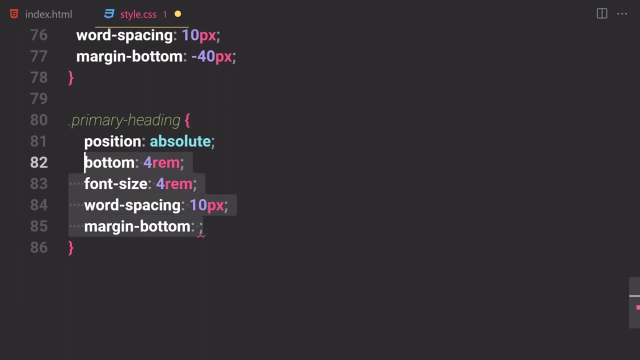 and what else do we got to do? we are going to be using the font size of forum. we want to increase the font size. now, let's just do the word spacing of 10 pixel in here. now, let's just provide a margin of bottom. okay, so we already write that style. okay, my bad, my bad, uh, what do we have to do? we have to. 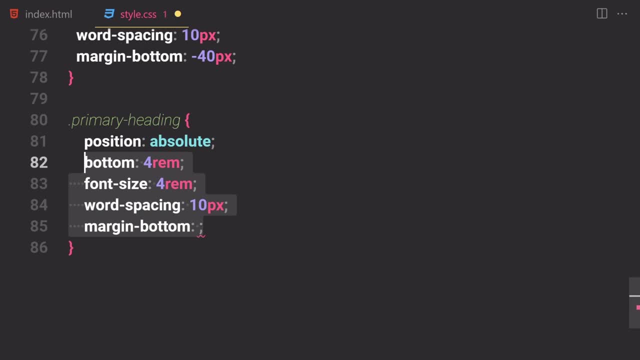 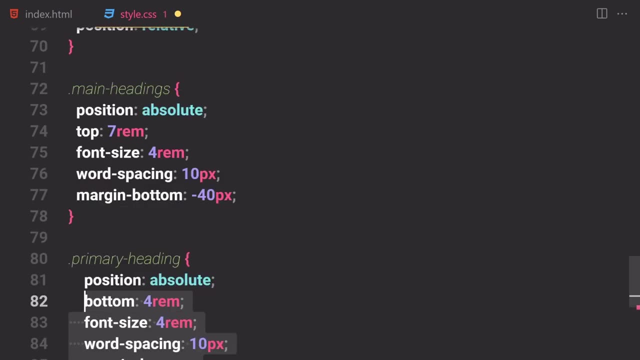 select, or yeah, everything is cool, but you know what? i did, mess up something right here. so for, uh, main headings, we have to write a position of absolute, we have to write a top and then font size. we don't need these. uh, world, world spacing owner. okay, we do need that, but we don't need that margin bottom. so if you, 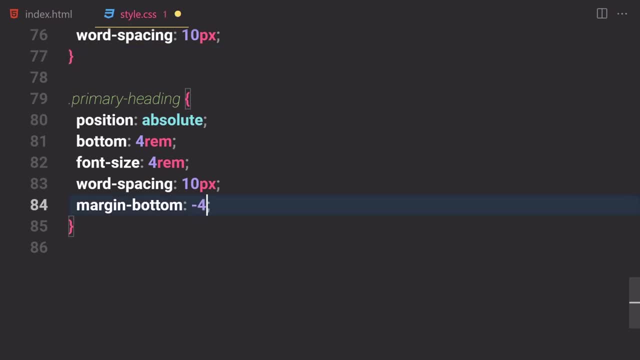 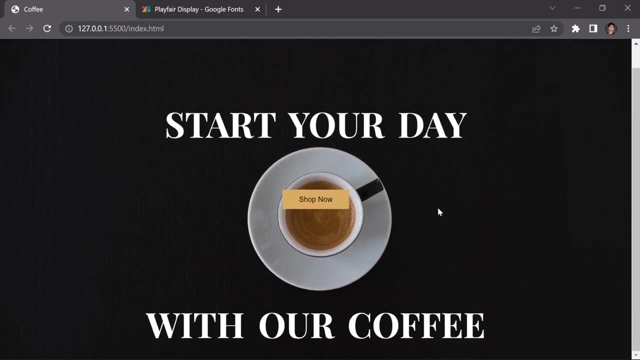 save that and finally, we just have to write the margin bottom right here like 40 pixel. so now, if you save that, and this is how currently things looks like, so now let's just take care of this button and then we are going to be at the good chip. so, uh, what was the class we gave to that? 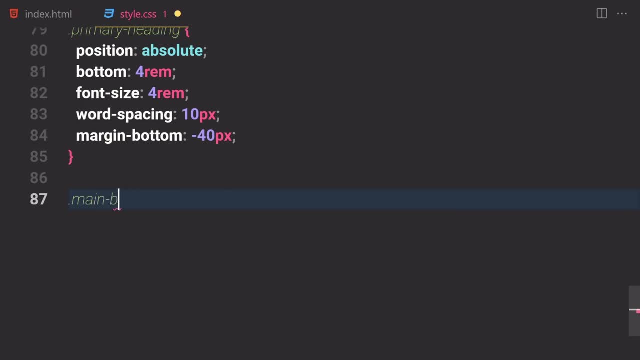 button, which is that main button. so now let's just select that real quick. so i'm going to select that main btn. and now let's just create a user matrix, and then we're going to get the moment that we'll going to create a user matrix and then we're going to get the moment that we'll 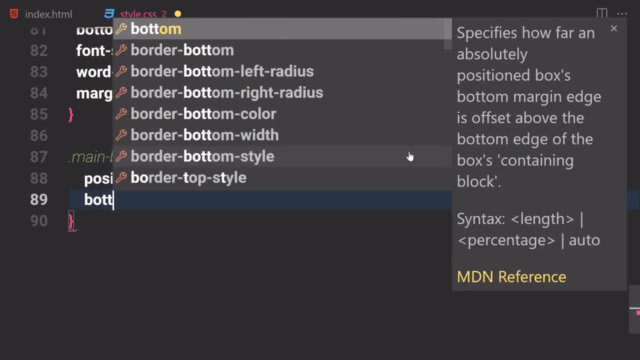 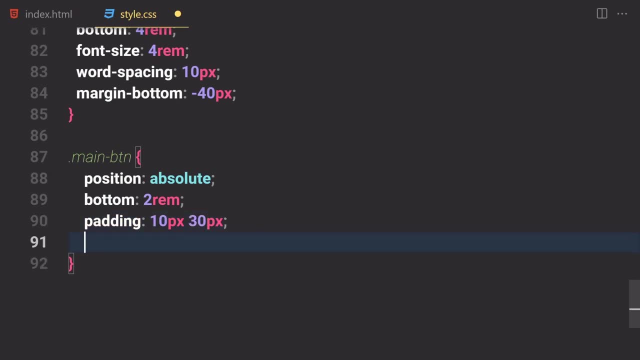 just use a position of absolute on a and a bottom value will be 2 rem padding we are going to be providing is like 10 pixel for the top and bottom and 30 pixel for the left and right, and now let's just use that margin top of 20 pixel. and now let's just change their background: not bottom, but just. 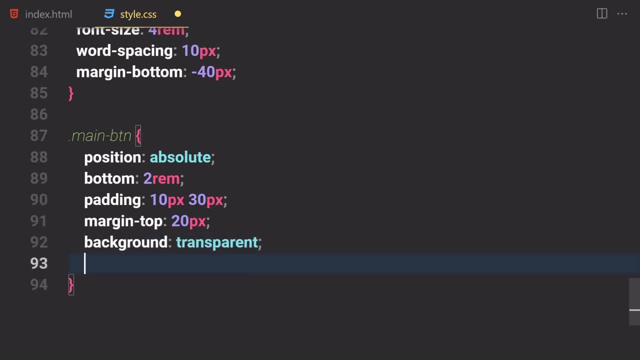 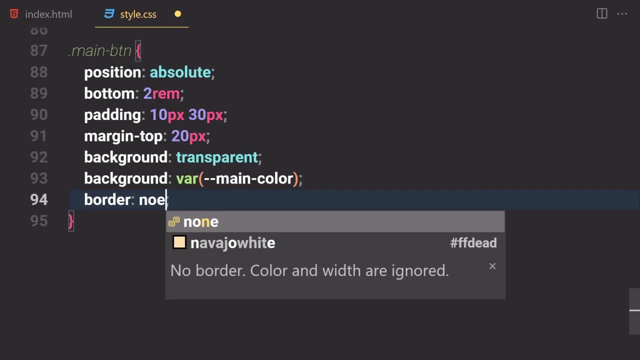 a background to be totally transparent. okay, and now let's just use the background color of that main color which we already declare, and the border will be also none, because we want to remove that border, and cursor will be already pointer. you know what? we don't need these properties. i'm going to 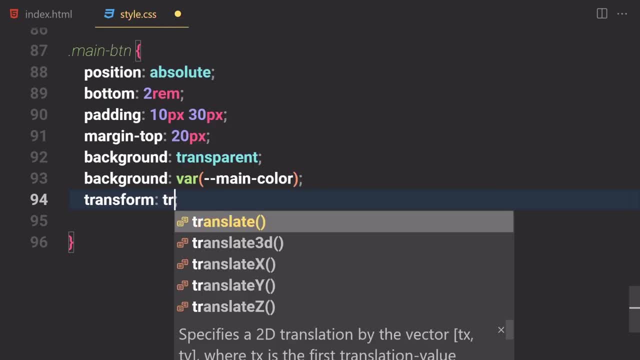 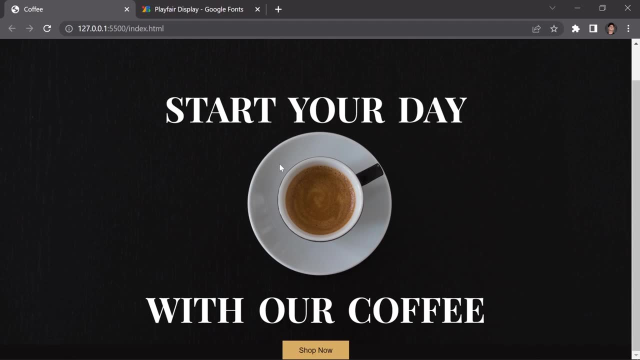 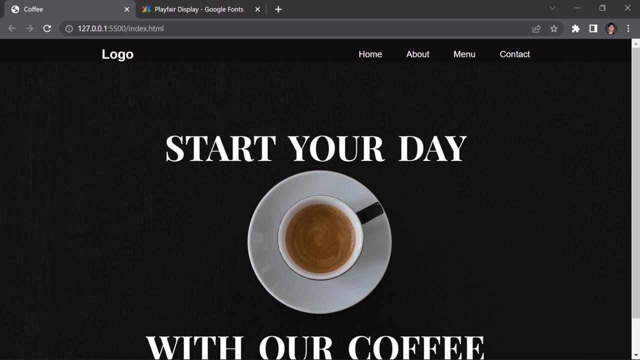 remove them, because we already write that and transform or translate it to the y axis, and here we are going to be providing a positive value. so if you save that- and yeah, it will excuse me- it will now push it to the bottom right here. so this is how currently or header area looks like. i know. 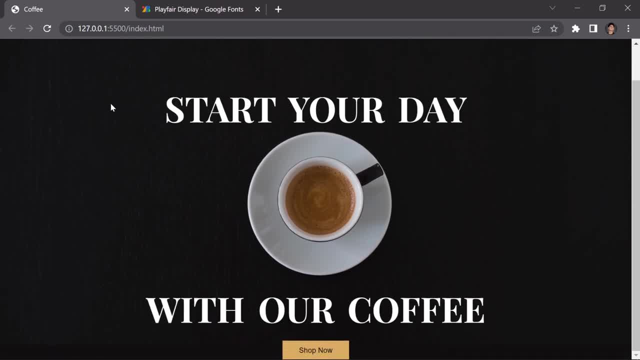 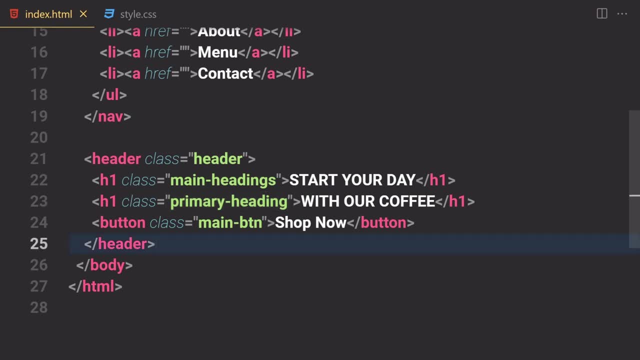 you really like their hair, you, and now we are totally done with this header area right now. so now let's just take care of that um or story and all of that kind of stuff. so what do we have to do here? we are going to be doing is: 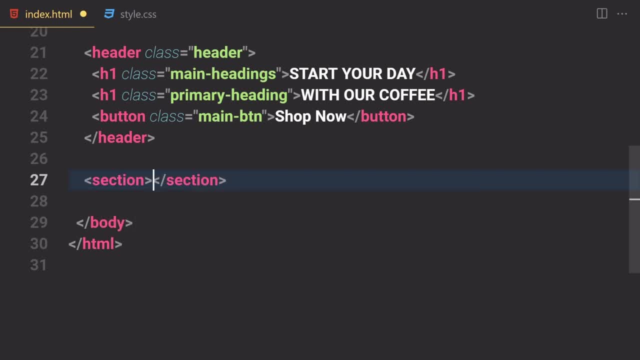 that first of all, we are going to be creating a section with uh id. i'm going to just provide id specifically or story, okay. so inside this id we are going to be just using a div with a class of image container. so this container will be for our image because we are going to be rendering. 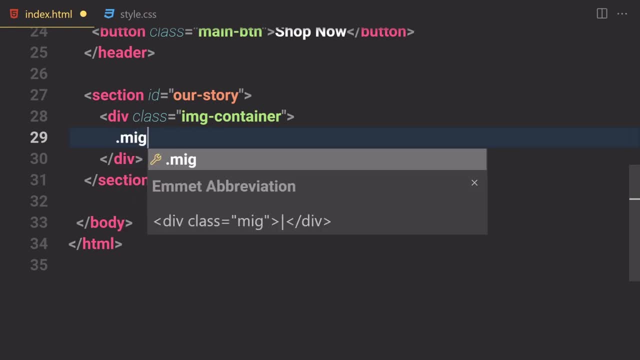 our image inside that container. so we are going to be using a div with a class of image container inside that container. so we are going to be using an img class for our image right now. okay, so we are going to be using a display flex on this one, and this is our first item. and now let's just write. 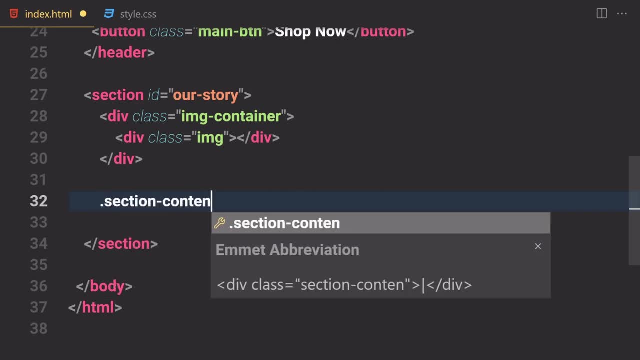 our next item, which will be a section and content content. inside this section- content- we are going to be using our title style first of all. okay, we need to write a style, and now let's just write a span for the line. so this is going to be your line, and now let's just write h1 with the class of it. 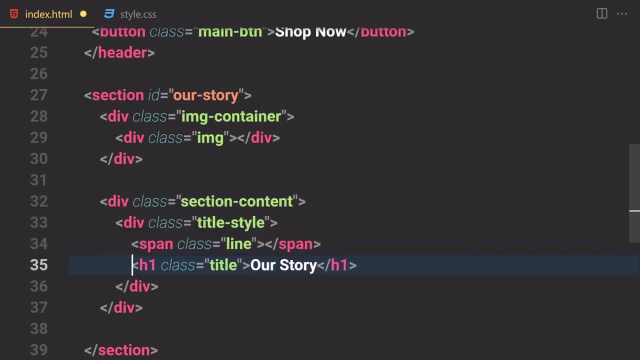 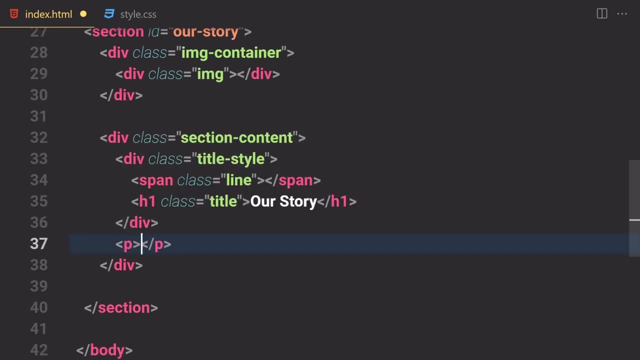 title, and the title will be or story, and so now we are totally done with this section. now, what else do we have to do underneath this div? we are going to be just using a p with a class with no classes whatsoever, so we are going to be just writing a lorem ipsum of whatever the text. 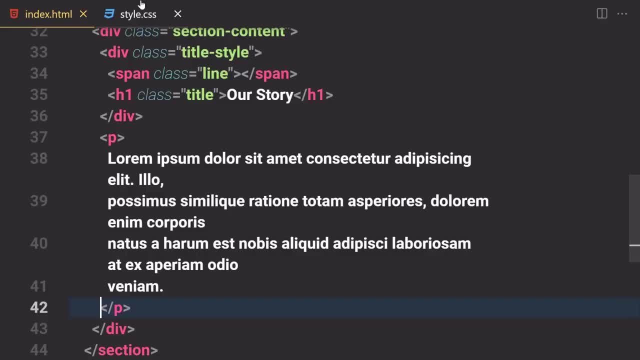 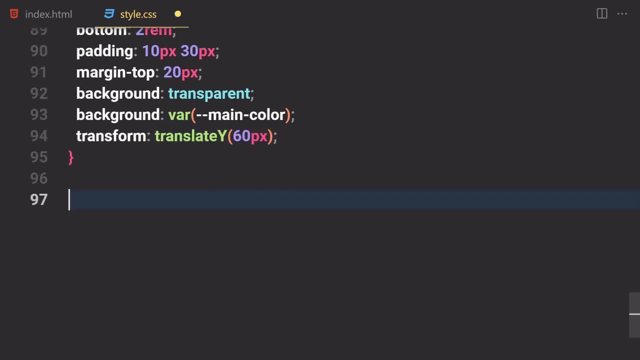 it gives us so cell file and we can all see that because we have to provide a height for it. so i'm going to just do that in a second. first of all let's just start working on or story section. so i'm going to just select or story by using a id selector. i'm going to give him a height of 100. 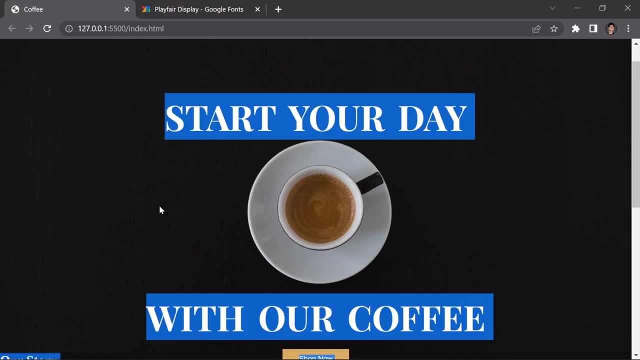 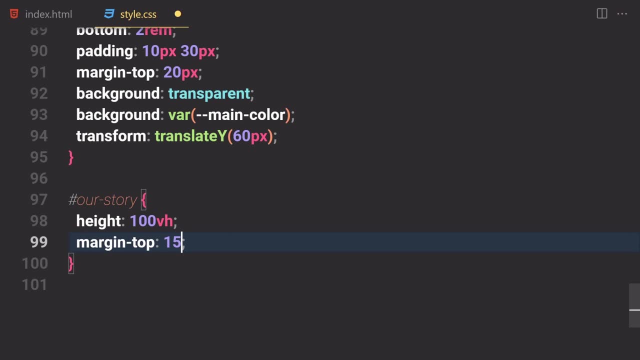 vh, so that we guys have a little bit of space, so that we can see everything a bit clear. all right, so that's for the height. so now let's just write a margin of top of 15 percentage and now let's just use that display flex, because we want to center everything, and flex wrap in this case. 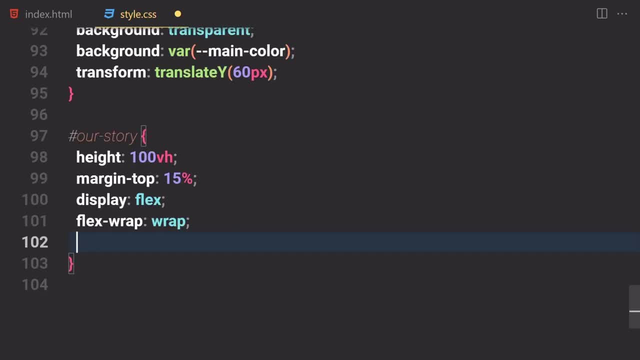 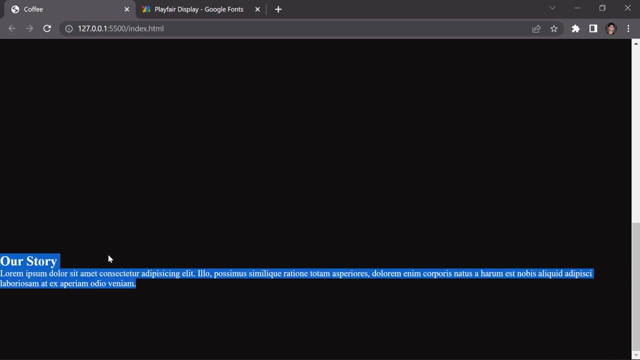 will be also wrapped, because we want our items to wrap for responsiveness reasons. so let's just justify content, property or space around, yet let's just use align items of center, and in this case as well. so, if you saw that, and yeah, here you can see, we have all of this text right here, but we cannot see it clearly. 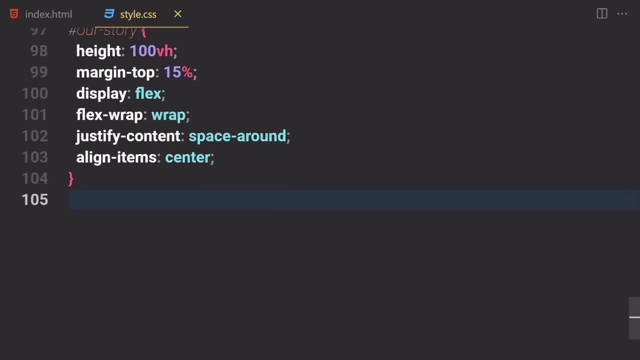 because for that we would need to provide a color and we don't want to do that right now. so what else do we have to do? we have to select this img right now and provide our image in it. so we are going to be using img. let's just give a width of like 400 pixel, and also the height will be 400. 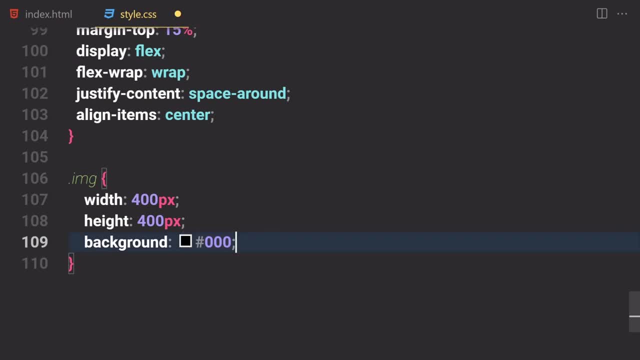 pixel as well. so now let's just use our background of url, not a color. so i'm going to just remove that and change it to like url and we are going to be going to our images and now let's just select this image right here. this second one: 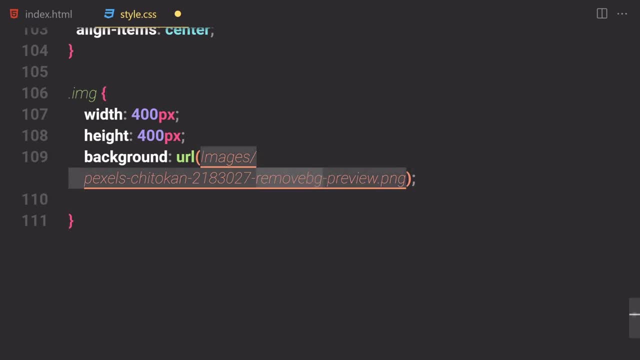 and uh, you already noticed that i'm using uh, remove bg, which is a soft which allows us to remove the background from our images and stuff. i'm going to show you that. maybe i'm not sure, but so if you just write a background position of totally center, and now let's just use a background, 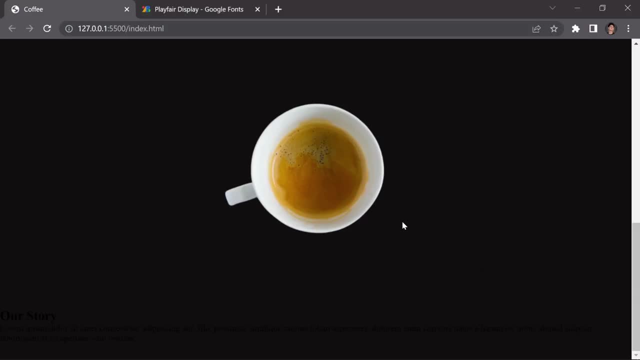 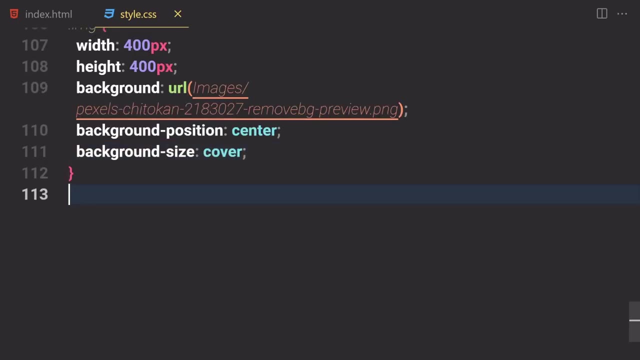 size of totally covered, so not contained but covered. and if you sell that here, you can see we have our cup right here filled with tea. all right, so now we have our image right here. now. the next thing which you have to do is that we have to start to styling this- uh, style. 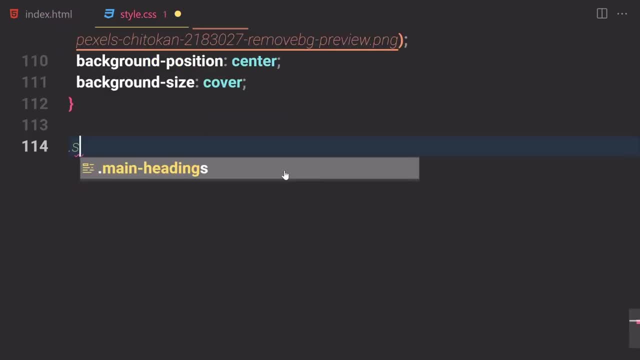 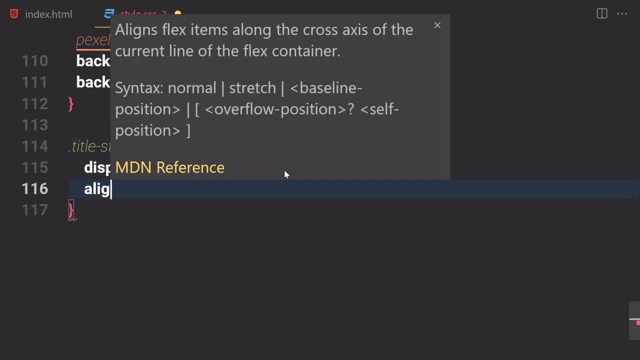 um, title style to be precise. so i'm going to just get there real quick. i'm going to write like a title and style and i'm going to just provide a display of flex on it, and now let's just use align item software center in if you sell that. okay, we cannot see that. i don't know. i guess i messed up. 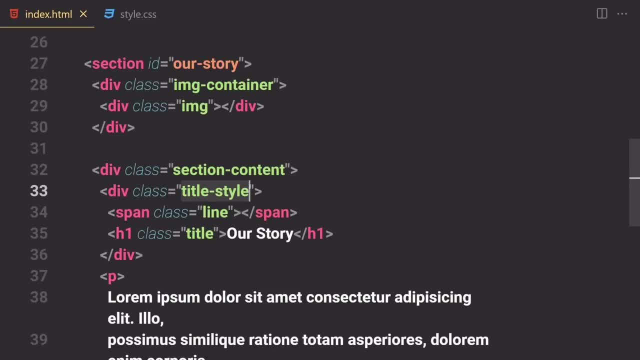 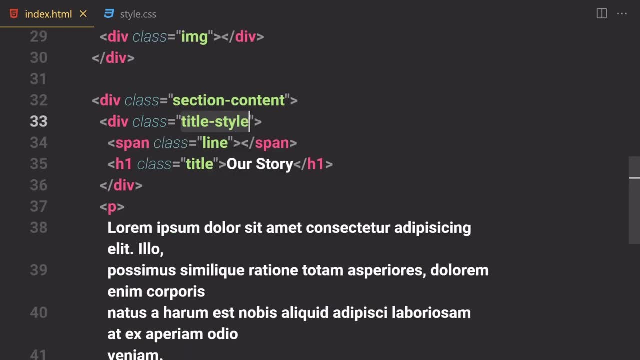 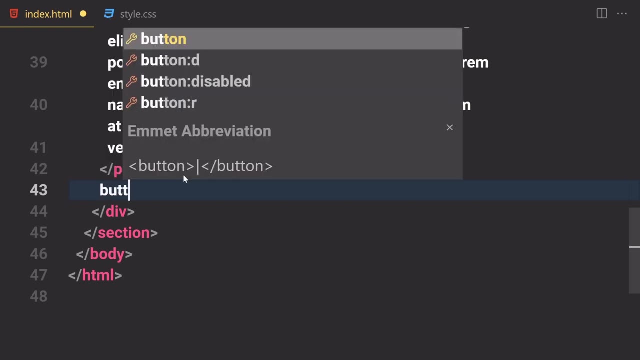 something in uh, html, html, i guess. so we have word story, then we have our image container, then we have our image inside there, then we have our section content, then we have title, style, line, tile and finally we forgot to include a button outside from this paragraph. so we are going to do that just in a second. i want. 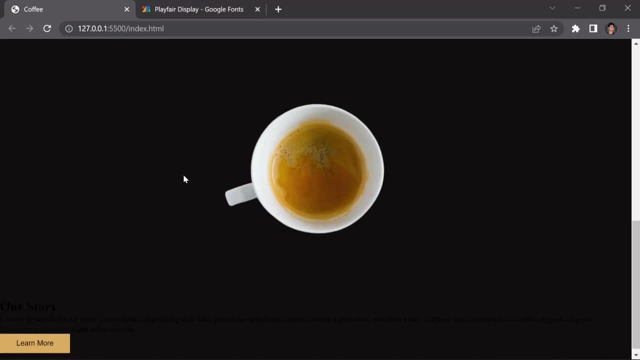 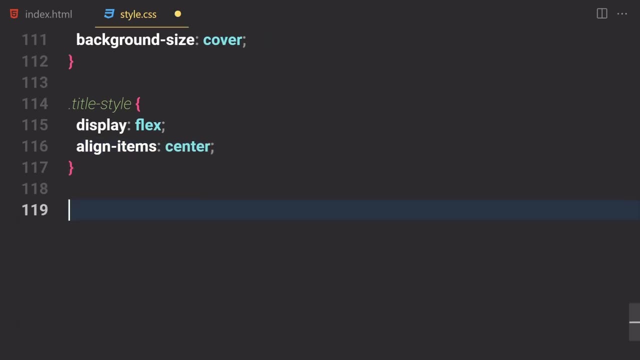 to just put like a learn more in it, and now, if you save that, we will get our button right here. all right, so this is going to be it for the styling of that title. now, what else do we have to do? we have to get a specific title which is: 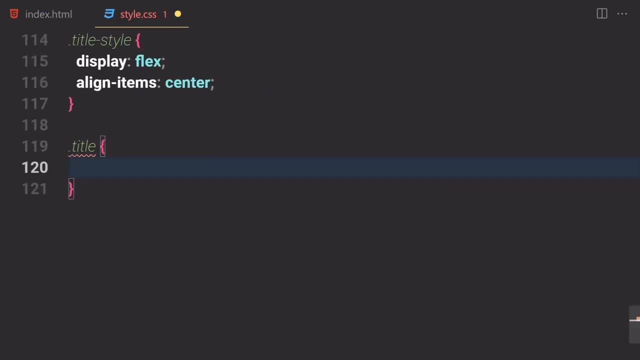 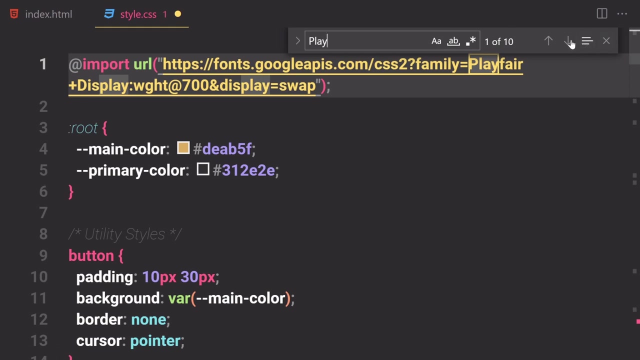 their title right here. so now let's just get there. and now let's use our font family. uh, oh, my goodness, it's not helping me, i don't know. okay, i just wrote a phone instead of a form. one family will be that font family which you just copy of play fire display. let's just search for that. okay, this is. 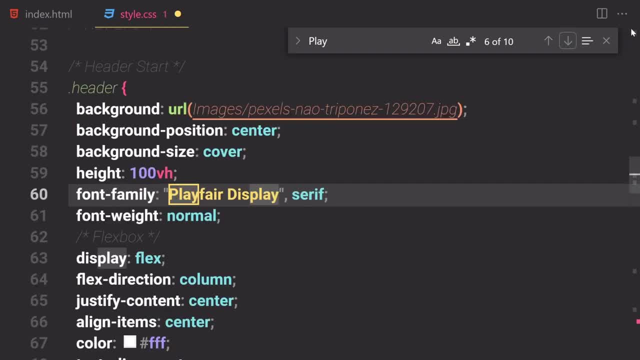 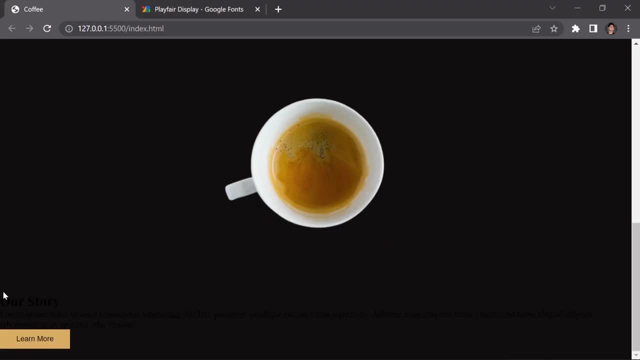 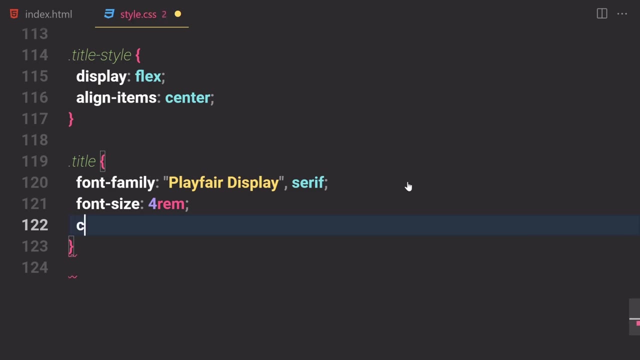 the second or third one. okay, we have display. yep there we go, copy that and go to the end and paste and you can now see that real quick. what else do you have to do? we are going to be using a font size of 4m and we are going to be changing the color to be totally white and also the 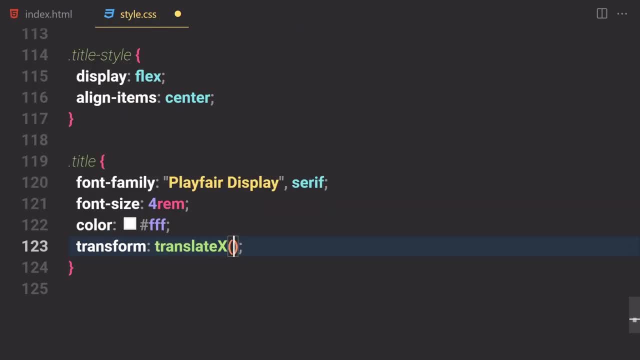 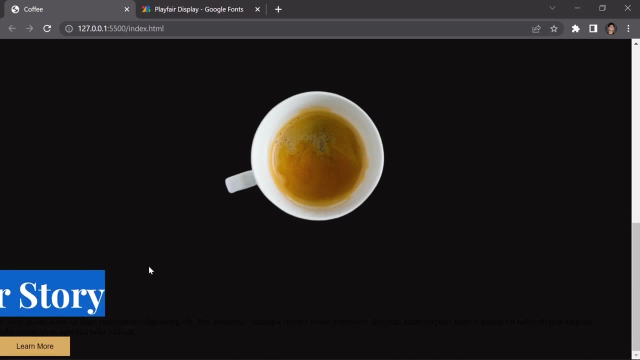 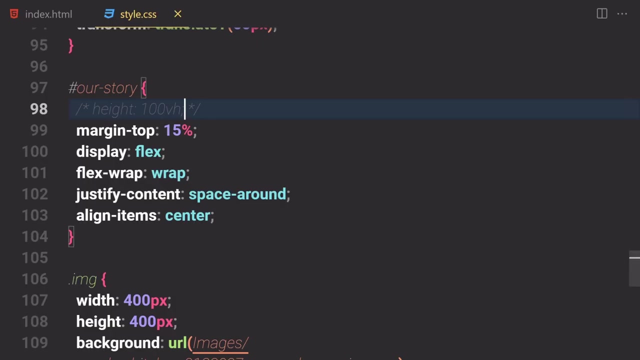 transformation would be like to translate to the x-axis. so we are going to be using minus hundred pixels. so if you sell that and you cannot see that that much clearly- but you will see that just a second- you know what? i'm gonna have to comment this line out. okay, okay, so. 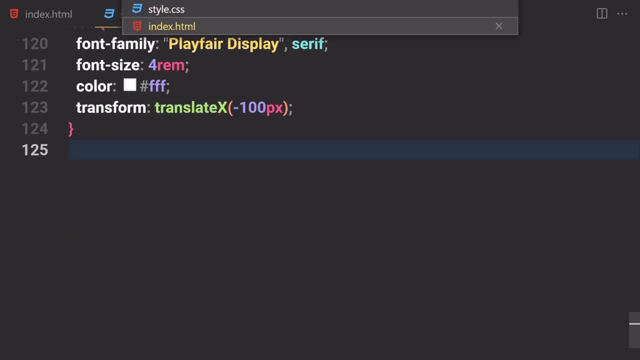 fine, now let's just start working on that line which we create right here, so we have that span with the class of line. now let's just select that real quick. i'm going to select that line and provide a width of like 100 pixel, and also the height will be 2 pixel. uh, yeah, 2 pixel will. 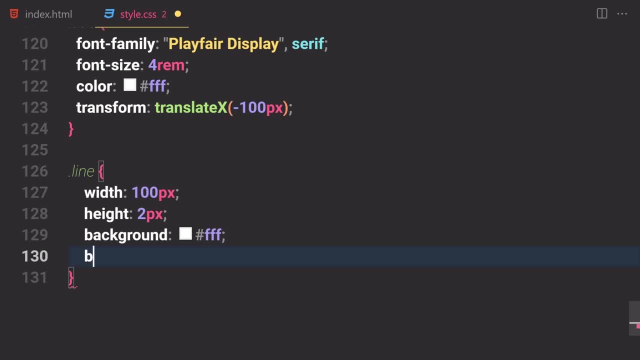 be fine. and now let's just use that background of totally white color and let's just use not a background color but a transform of the translated to the y-axis- not a y-axis, but the x-axis. and now let's just use 120 pixel, and if you sell that, and this is how our line looks- 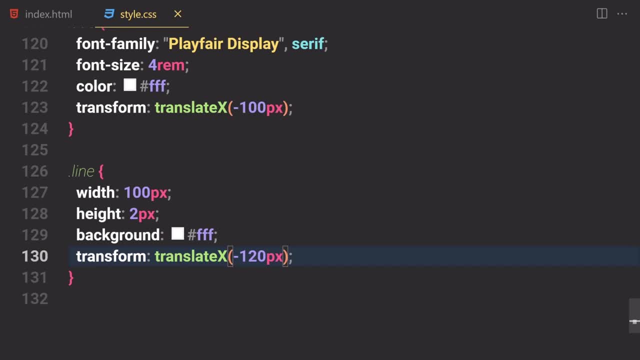 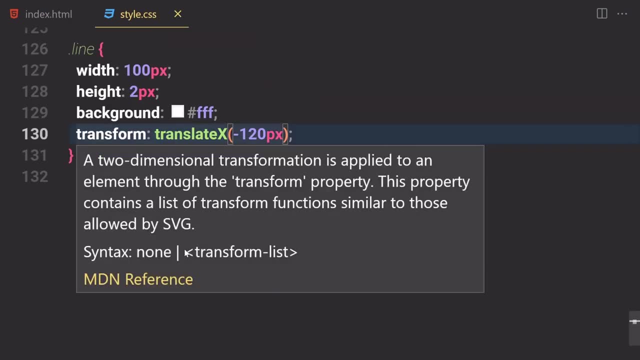 like, but you cannot see that right away. you'll see that just in a second. now let's just start working on our paragraph. so our paragraph is looking totally awful and now let's just style that a bit. so what do we have to do? we have to first of all select our section content, which 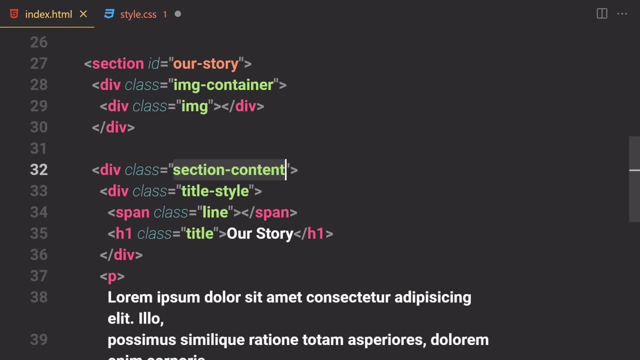 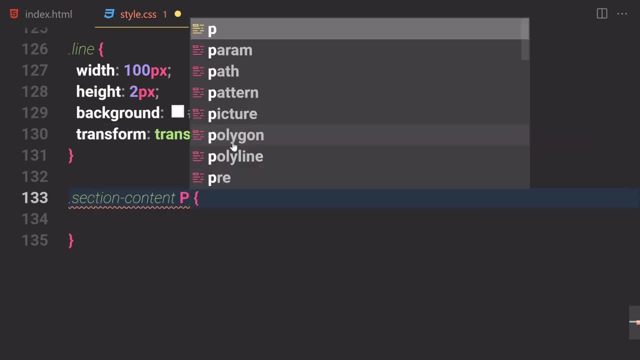 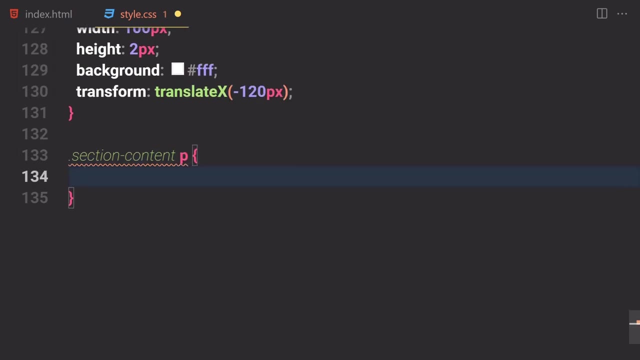 is that section? uh, content? let me just grab that. i guess i misspelled it in my css. grab that, and and and and pasted in here. all right, so now let's just select our paragraph right here. oh my goodness, what's wrong with my keyboard. let's just select that paragraph in there. and now let's just provide a. 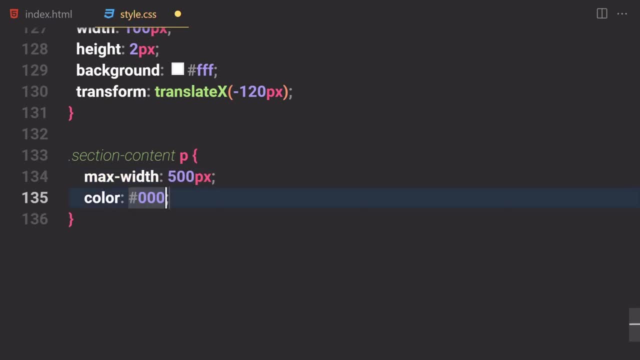 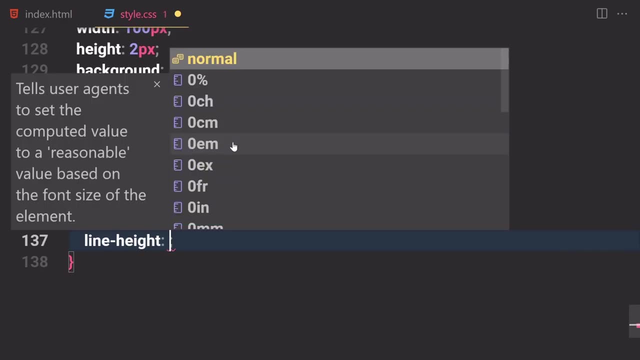 max width of like 500 pixel in this case and the color will be totally white, and also i'm going to use a font family of sans serif in this case. we don't need that play fire display or play fair display. line height will be 20 pixel and margin will be 20 pixel for the top and bottom and zero. 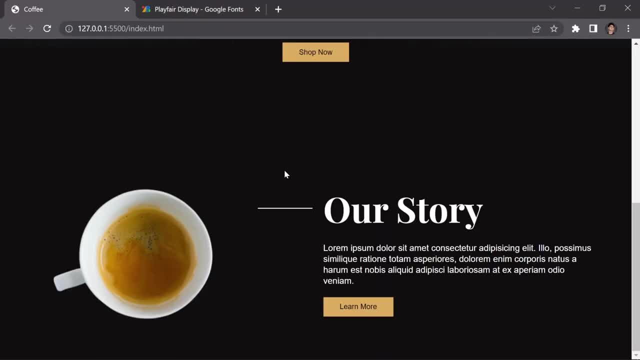 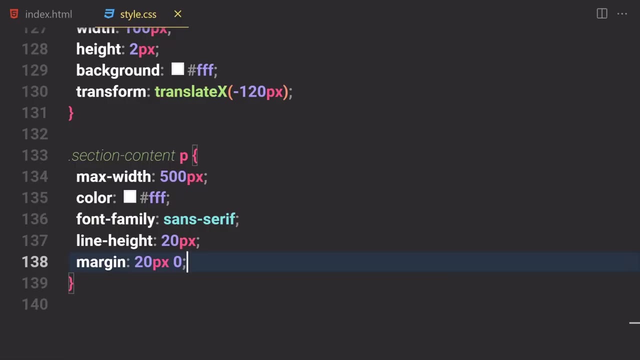 for the left and right. and now, if you save that- and yeah, this is how it looks like, so we are now totally done with this section as well- so you can increase or decrease the sizes if you want to, and this is our line, this is our story and this is our header area. this is all. or story area, right? 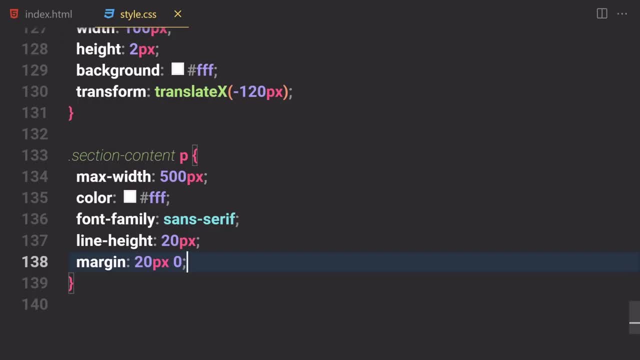 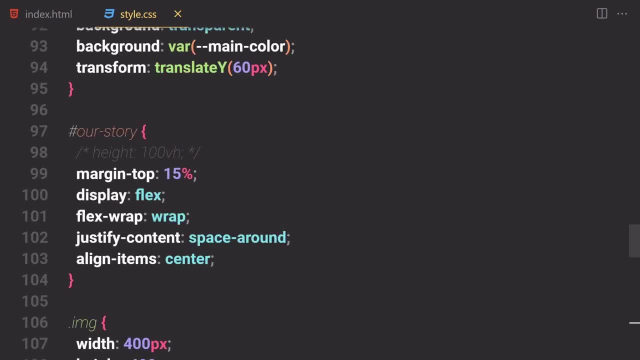 here so you can play around with the styling. but uh, i guess that would be fine for me and i wrote a comment for myself. i guess, or data and i, you have a man headings, then we start working you on our story. but i forgot to write a comment for myself, so i'm going to just write like: 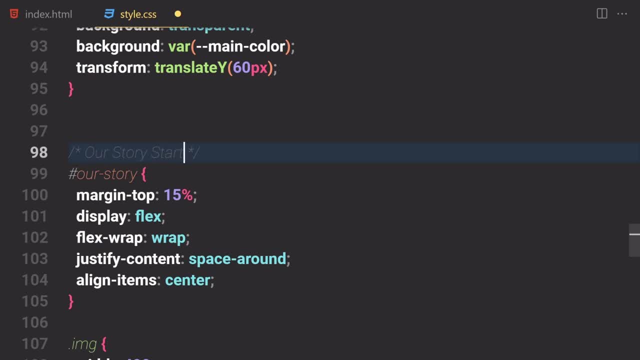 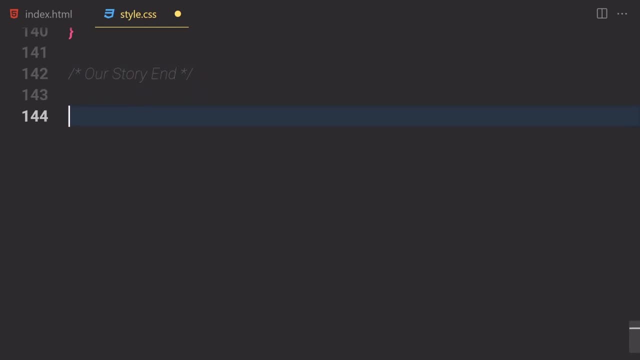 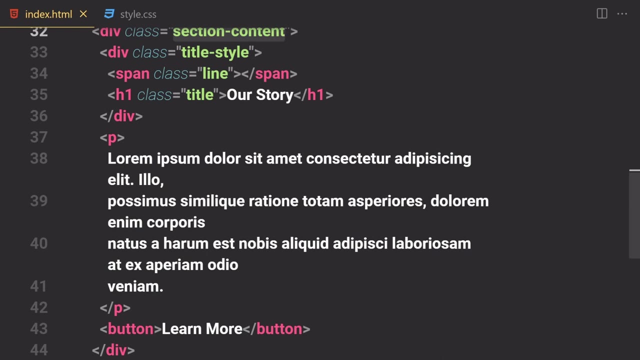 or story start, i'll just go to the end, and here i'm going to just write: uh or story end. okay, so now let's just work on our new section, which is called that coffee container section. so now let's just work on that real quick. so inside my html, outside from 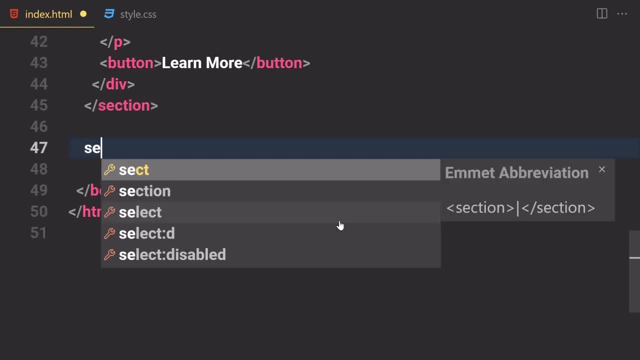 this section. what do we have to do? we have to create a new section with the class of coffee container section. so now let's just work on that real quick. so inside my html, outside from this section, what do we have to do? we have to create a new section with the class of coffee. 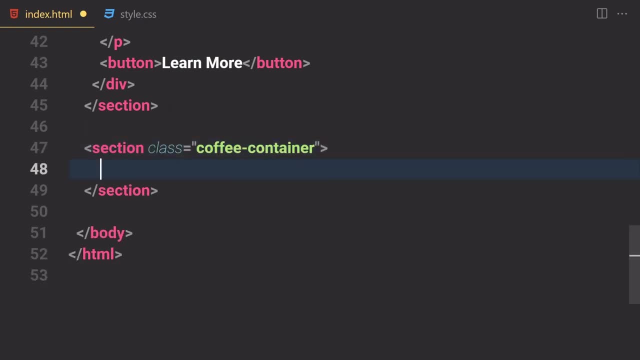 container, container. i know it's long, but you have to remember that now, inside this coffee container, we just have to write a content section. and inside this content section, what do we have to do? we are going to be first of all writing our title style right here inside. there we are going. 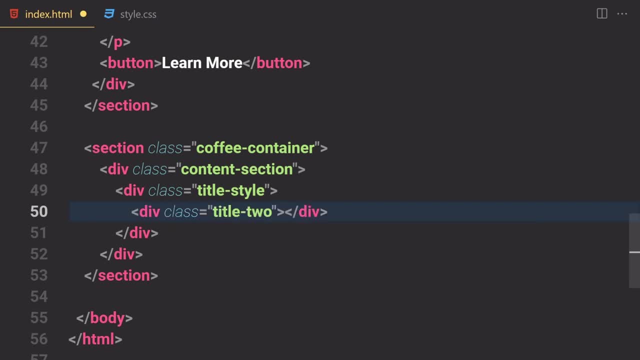 to be using a new div with the class of title 2.. this is going to be our second title and now, inside this title 2, we are going to be writing like a perfect place, and then br for breaking. and now let's just you know what. we are not going to be duplicating that, i want to be duplicating the. 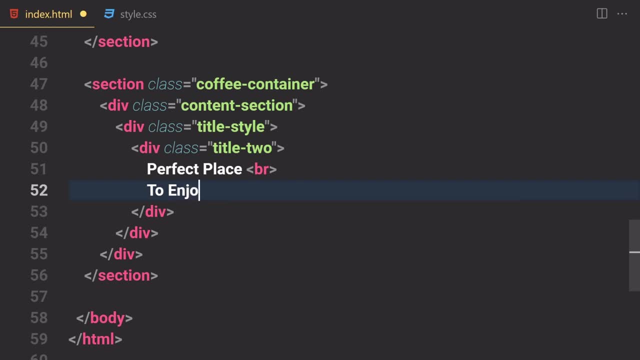 i want to be duplicating that. i want to write every single thing. so to enjoy your br and coffee. let's see, oh, double f, double e, okay, so outside from. okay, i messed up something. uh, it shouldn't have to be a div, it should have to be h1. this one will be also h1 and i guess we are fine. so 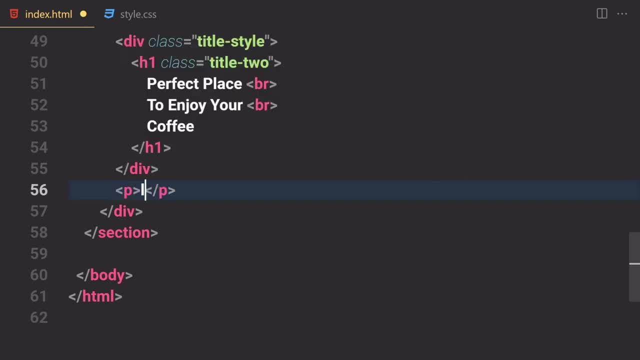 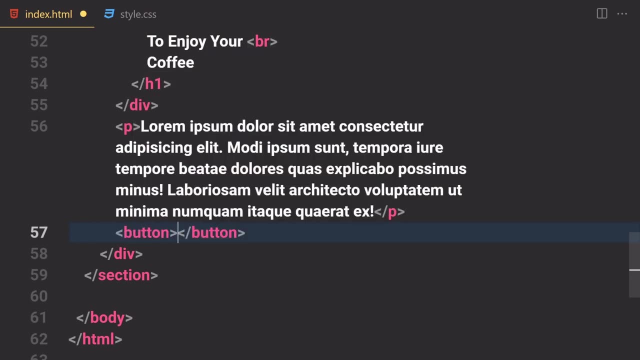 outside from this uh, div. right here, we have to just write a paragraph, the class of lorem, inside there and outside from this lorem. we are going to be using a button right here and i want to just put like, uh, i don't know. i want to put like: learn more in this case and now, if you sell, 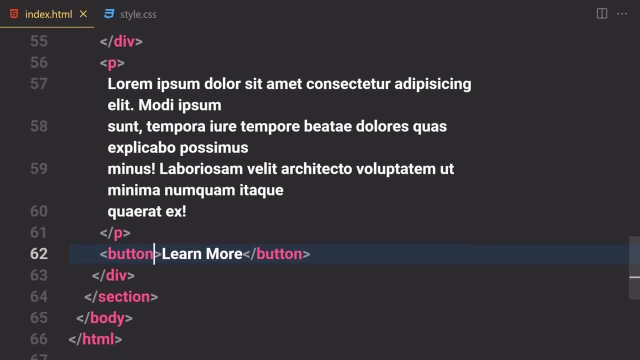 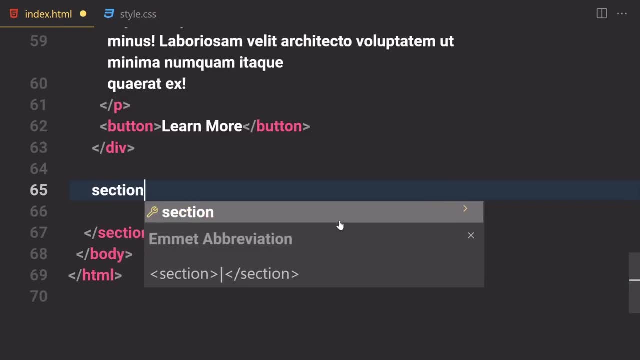 file and now we are done with this section. but we also have to write a little bit of code for image and container and stuff. so outside from this div, what else do we have to do? we have to create a new section with a class of img container. okay, so now inside this image container, we have 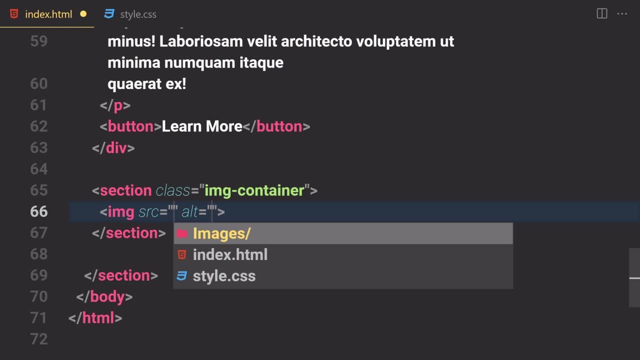 to render that image which we have somewhere. just hit control space, go to images and select that second image right here and as alt text. so i'm going to just give like: uh, i don't know, you know, i'm gonna not, i'm not gonna be putting any alt text, i'm gonna just 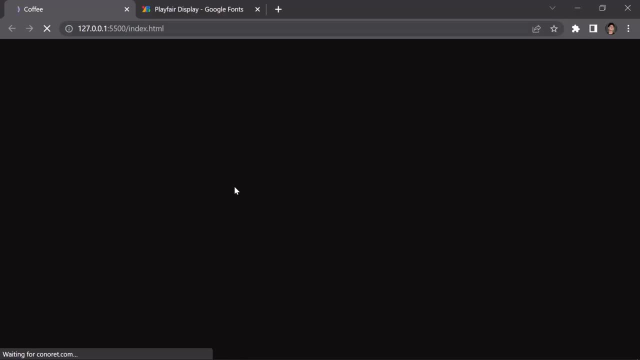 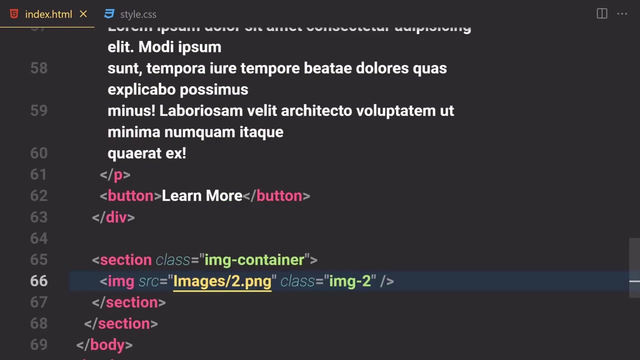 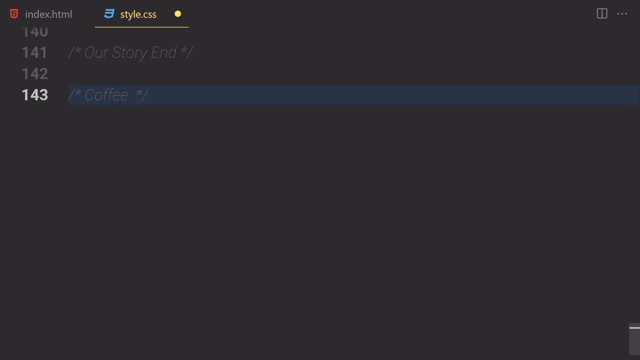 give a class of img2 and server file, and this is how currently things looks like right now. i know it's messy and long and stuff, so now let's just work on this section. first of all, we have to go to our css and now let's just write: or uh, coffee, uh yeah, coffee star would be fine. 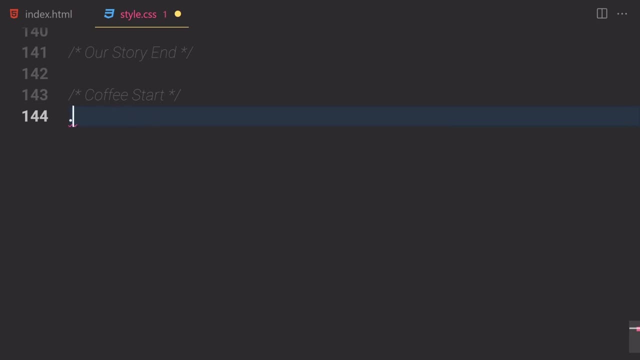 now let's just get our container- uh, not container, but coffee container, which is that coffee container which you wrote right here. so we have this copy container and we selected that. now let's just use our magic of display flex: justify. content will be spaced around in this case. 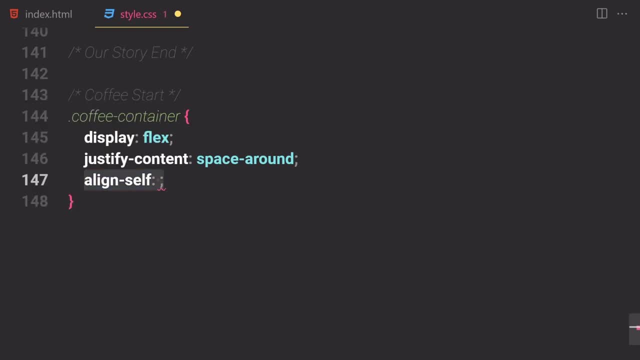 and we are going to be using aligned items of. okay, i just use align cell, so we have to use align items of. what align items of? totally center and i forgot to include something: card of flags, a wrap off wrap. so, if you save that. and i also forgot to include a margin top of 10. 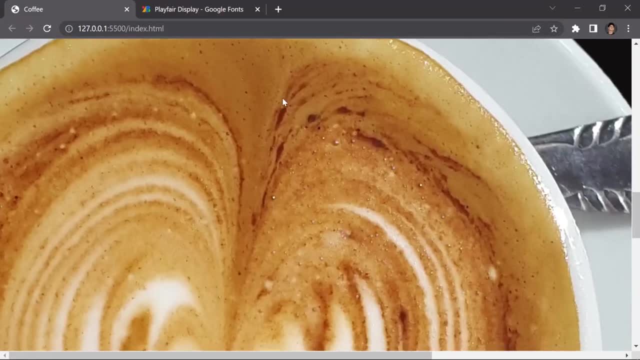 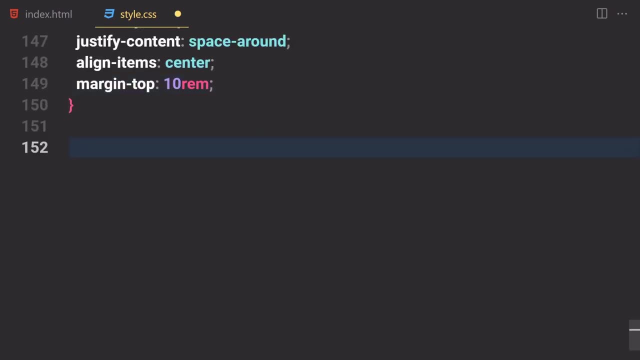 rim in this case. so we are going to be using 10 rim and this is how currently things looks like. so now let's just get into that image container and provide a little bit of width and height for that, so you guys can see everything a bit better. i'm going to just select that image 2, i guess i 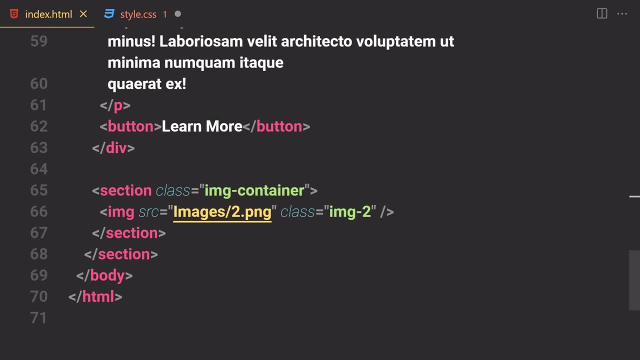 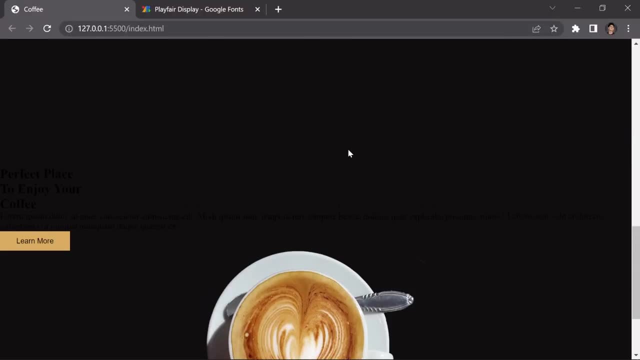 gave a class of image 2, yep, image 2.. i'm going to just provide a width of like 400 pixel and also the height will be 400 pixels. so if you sell that, and this is how currently things looks like right now. so now let's just 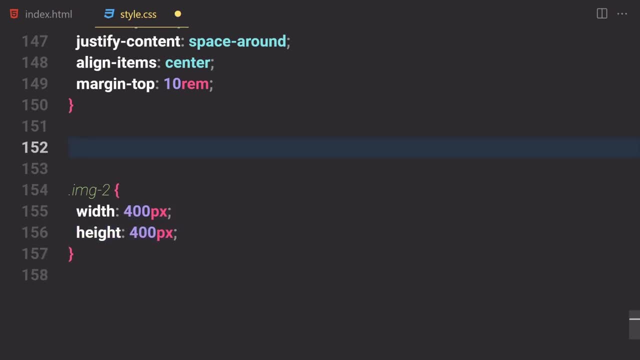 make it a bit better by first of all selecting or paragraph which is that paragraph. so we have a lot of content inside there and we can decrease that if you want to. so i'm going to just select my uh content section and now, inside this content section, we want to get our paragraph. 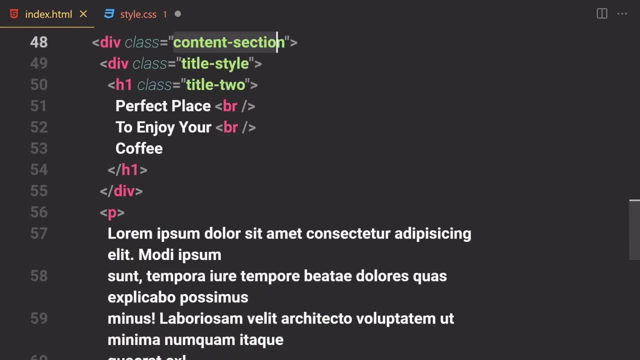 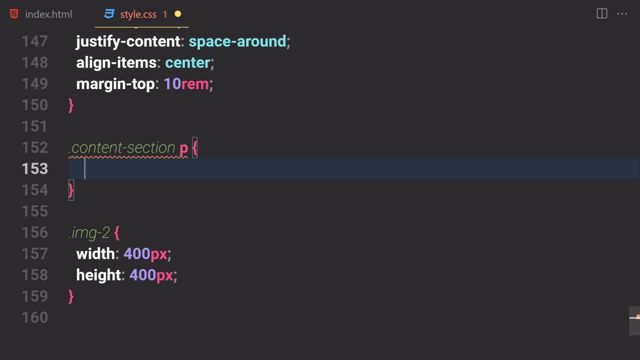 so we are now selecting our content section. inside this section, we just have one paragraph right here. if you have more than that, so we'll also select it there as well. so in this case we just have one paragraph. so we will now select that and i'm going to just provide a. 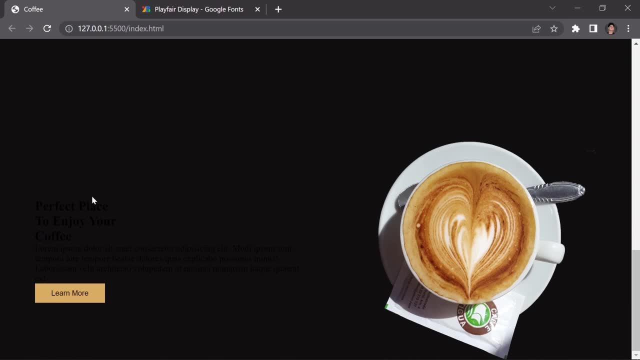 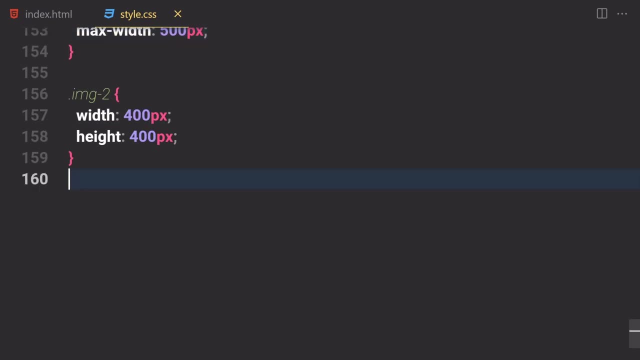 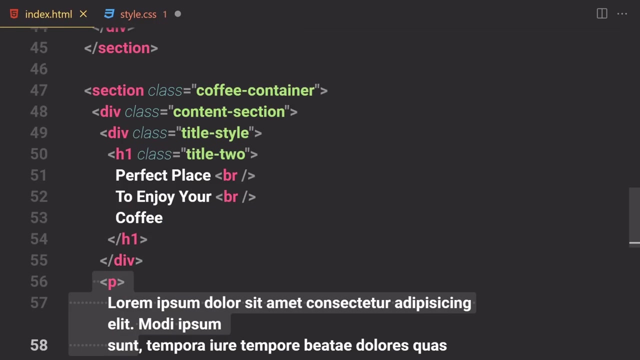 max width of like 500 pixels, and if you save that and it will just shrink it down to 500 pixel size right here anyway. so that's it for a basic styling. what else do we have to do? we are going to be selecting now in this case, or title two. so let me just show you that title two right here. so we have. 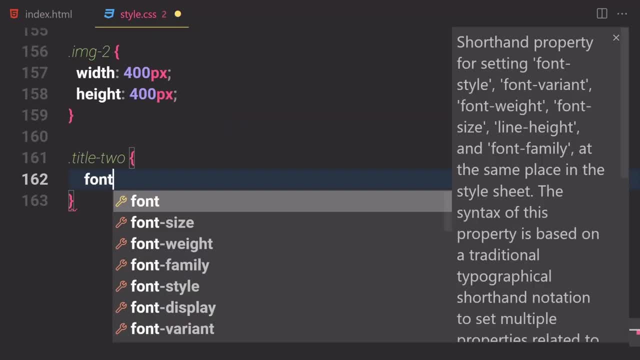 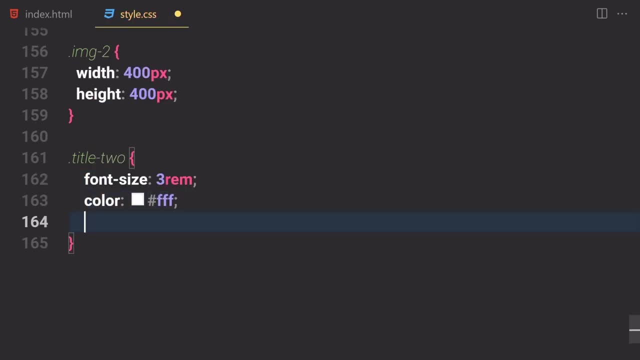 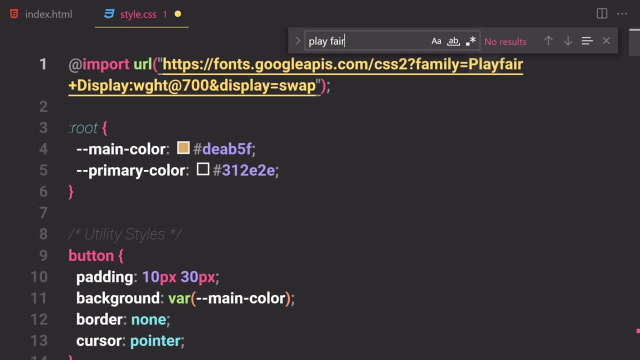 the title two. and now let's just use a font size of three uh rim right here. so the font size is going to be totally three rim and the color will be totally pure white. now let's just use that font family of play fire display. okay, play, go to bottom, bottom, bottom, bottom and bottom. here that's. 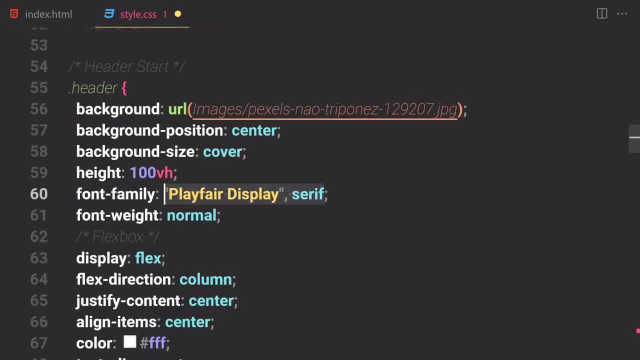 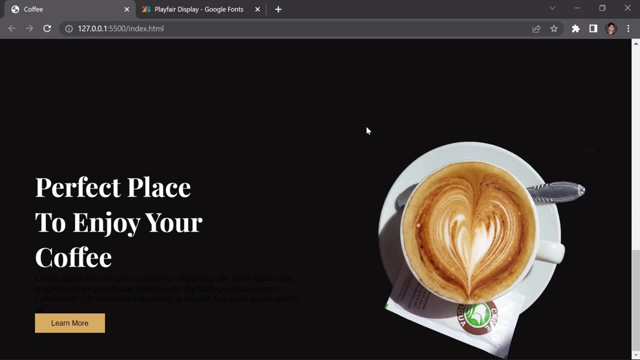 copy head and i'm going to paste it at the end. so i'm going to paste it right here and save file. and this is how currently things looks like right now. you know what? the font family is just a little bit huge, so i'm going to just save it right here. 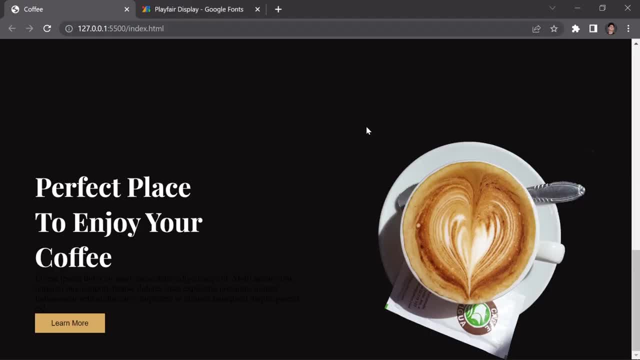 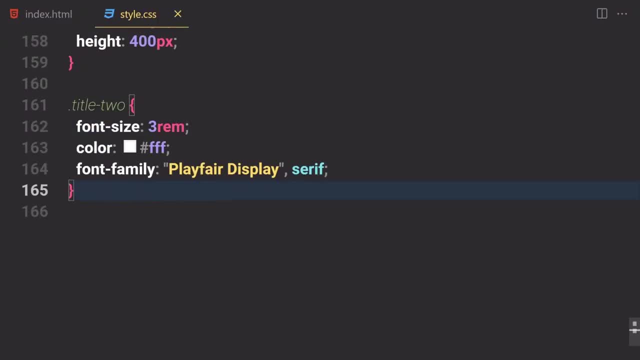 there too, i found a way to normal. so now, if you save that- and yeah, we just have one form family, so i'm going to remove this more family from there, i mean like far away from there. now, what else do we have to do? uh, we already select this. so you know, i'm gonna cut that from here and i'm gonna 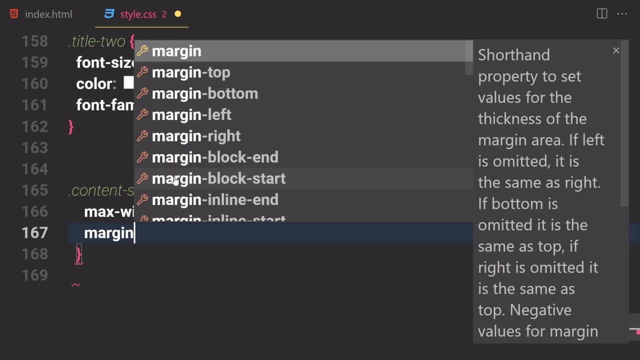 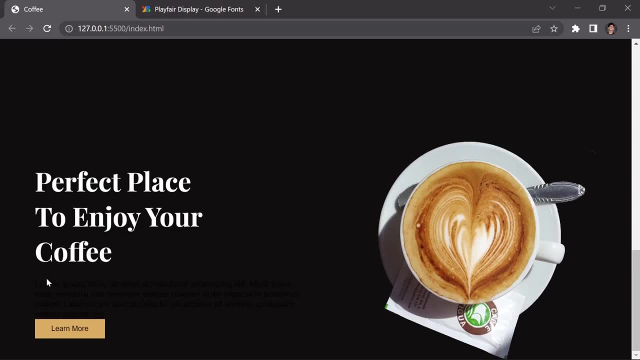 paste it right here and i'll just write like: margin of top of 20 pixel and form. family in this case will be just totally sensor. so save that. and you cannot see that because the color is totally blank. um, so i'm going to just write a c of colored and seven, and we have a lot more. 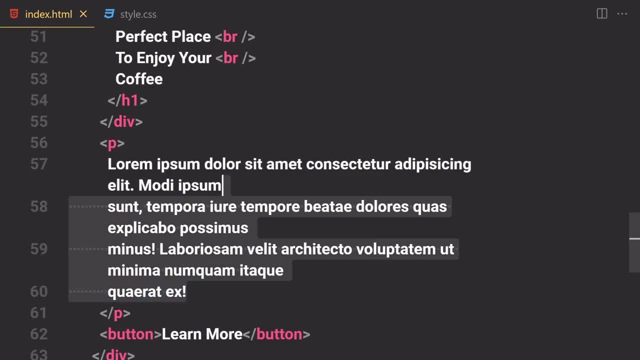 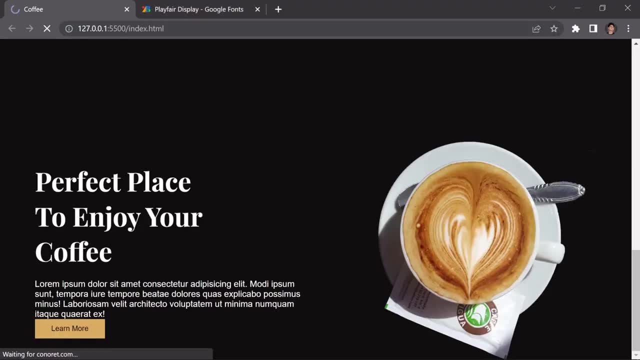 content. so i'm going to just remove some of this content from here. okay, not that much, but i guess that would be fine. two lines, you know what? all of them are fine, but i'm going to just provide inline style in here. i don't want to provide a new styling for this one, so i'm going to just write. 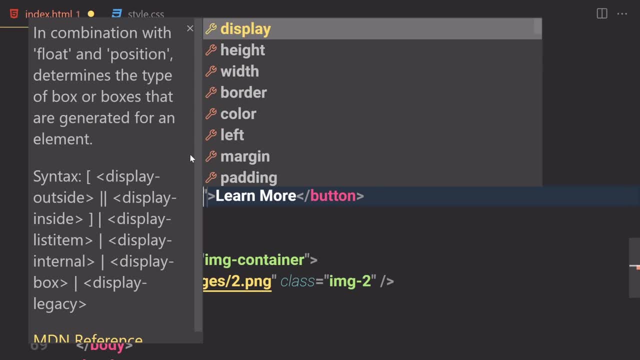 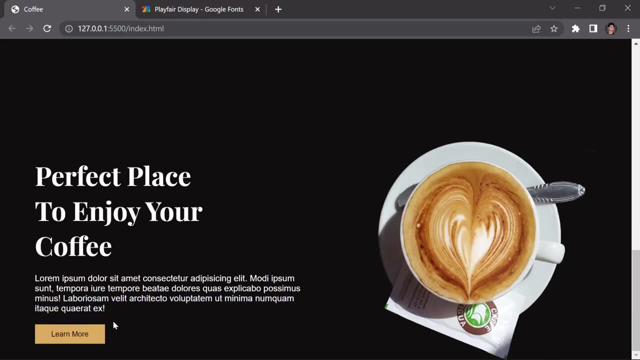 like style and let's just use inline style of margin top. let's just use margin top to be like 20 pixel in this case. if you save that, it'll not give us a little bit of margin in there. so we are not totally done with the header area. navigation- header area. 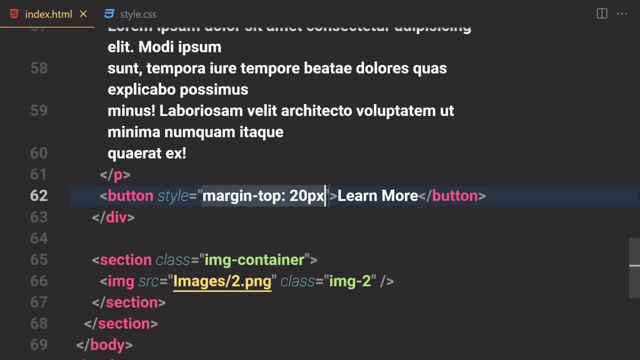 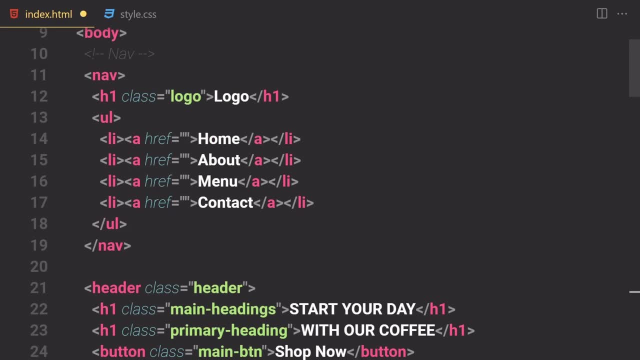 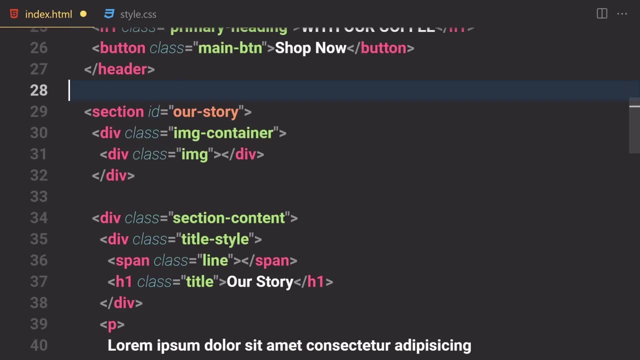 or story, and perfect place for a coffee and stuff. so now let's just work on our product section. so what do we have to do? i guess i didn't write any comments in html file, so we have a nav. then we have or a header, a header right here, then we have or story. 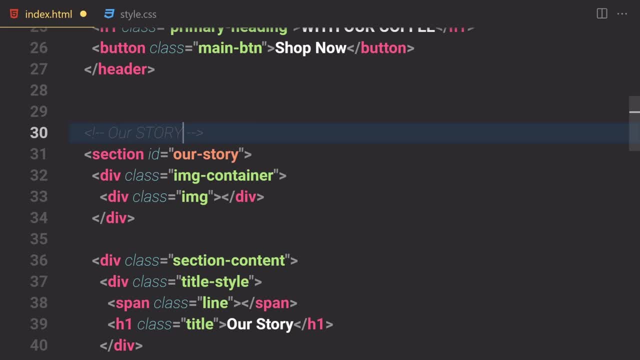 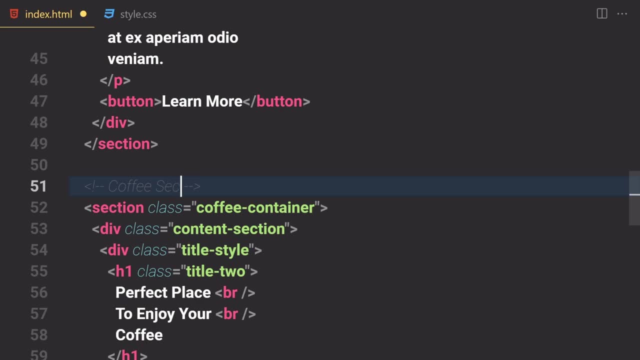 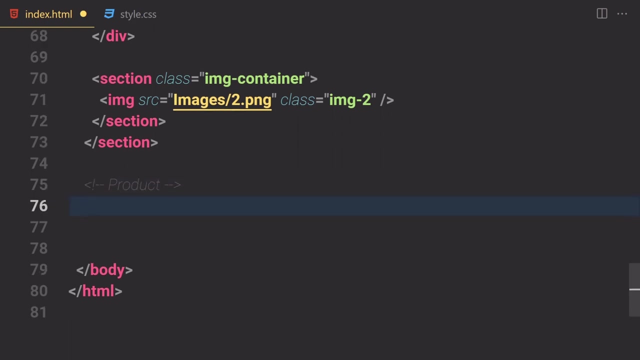 or story, and now then we have another one or story, then we have or coffee, coffee section, and now let's just work on a new section, which is the product section. so i'm just right like a product in here. so for this product section we have to first of all create a section. 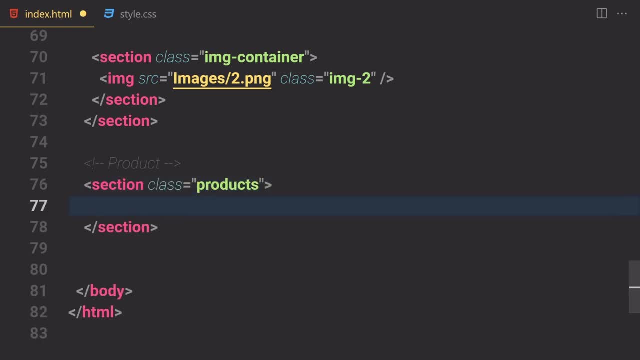 with a class of products inside this section. we are going to be writing over h1 with the class of title and another class of title three, because this is going to be our title three, and now let's go to our products in there, and now let's just create a section for our cards. so we are going 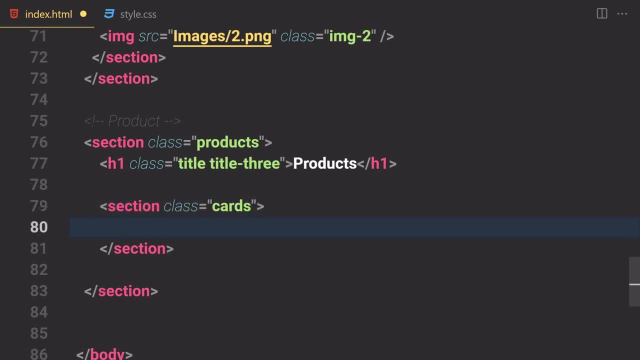 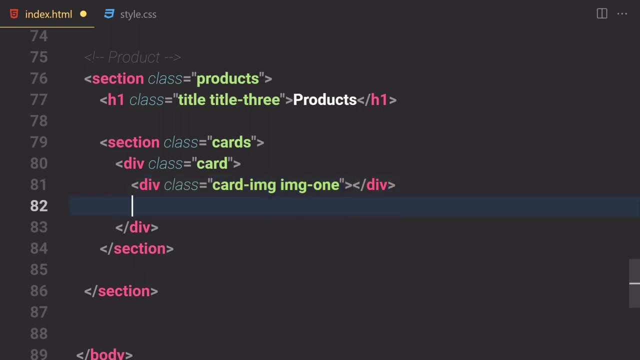 to be writing a section for cards and inside this card section we are going to be creating a few cards. so we are going to be just writing card one. and now let's just give a class of card, img, and then img one. so this is going to be tagging our image, and then let's just use our. 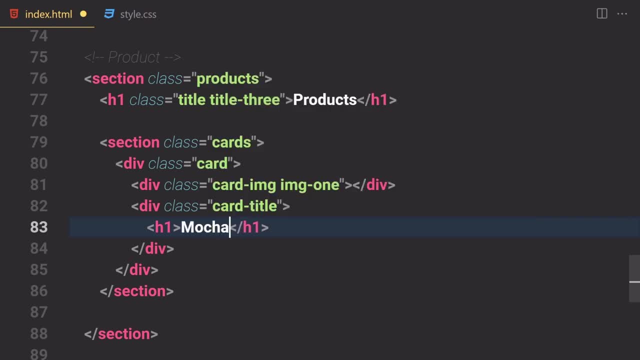 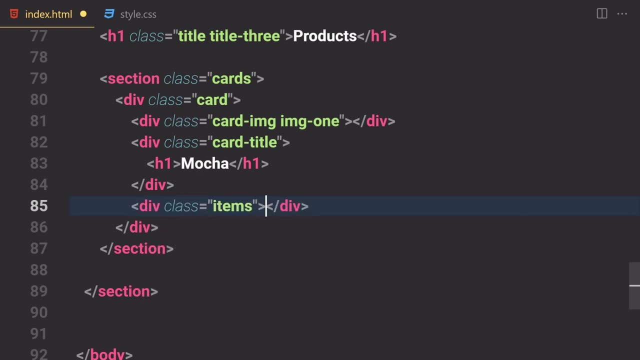 card title and inside that we are going to be using our mocha card. and now outside from this dev, what else do we have to do? we are going to be writing an items container, so this is going to be your items container, which will take a lot of four items. so i'm going to just write like, uh, different. 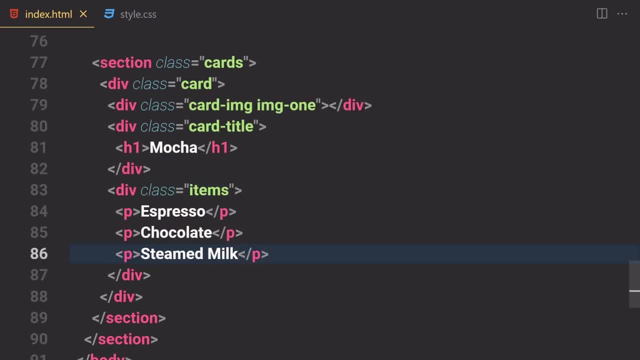 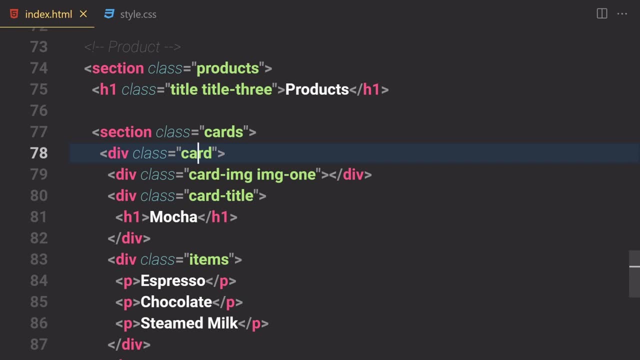 kind of names, all right. so now, if you sell them, and now let's just style that, and we are going to be duplicating that just in a second, but first of all we have to style that, and i guess something is wrong. you know what? first of all, we are going to be duplicate right here, so we change our style and 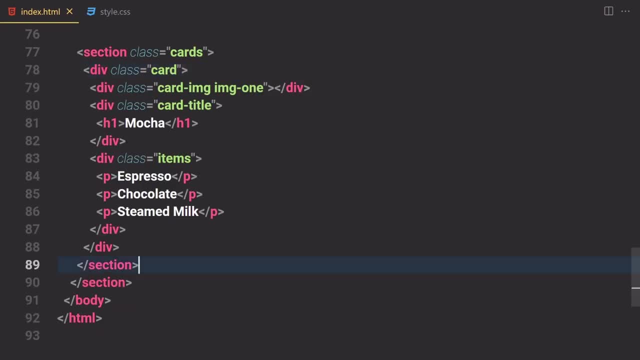 and you know what? first of all, we have the style there. there, simply say anything will, do you just not? let me just write all of the html code, then we will style that. so we have our card section right here. now we have to start, uh, copying from this area, because this is our first card. and now let's. 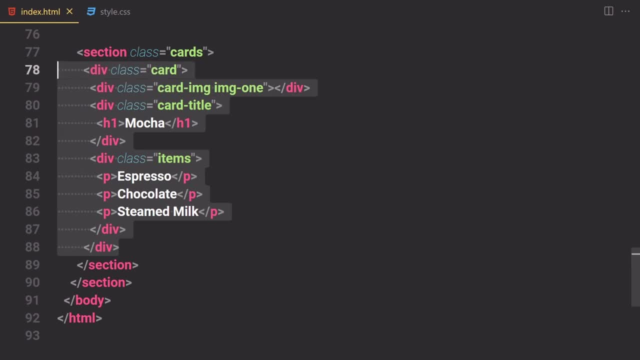 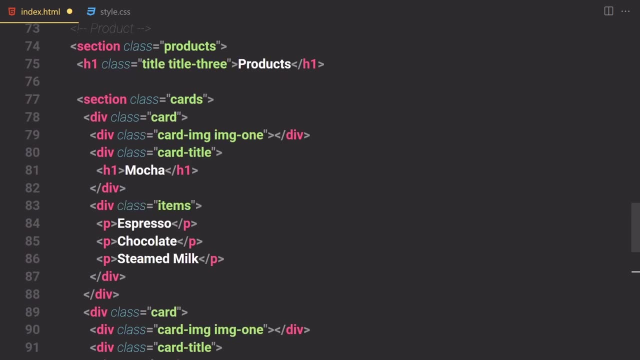 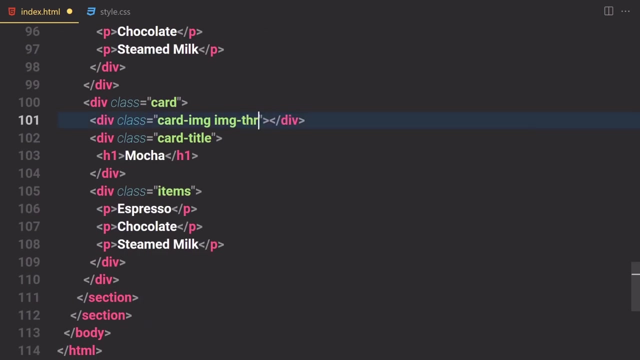 just start duplicating that. so this is our card one, and now i want to duplicate to card two. then we have our card three. all right, so now let's just change our stuff inside that. so this, or card image, card image one, this is going to be our card image two, and this is going to be our card image three. 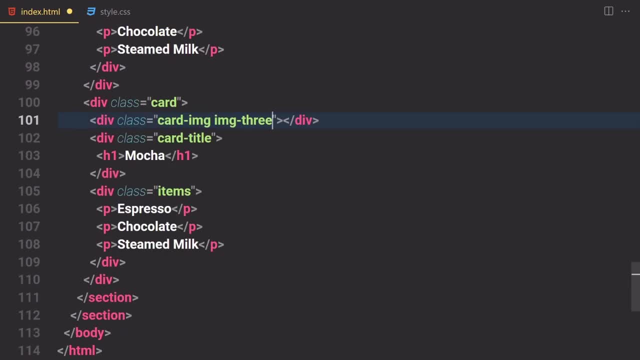 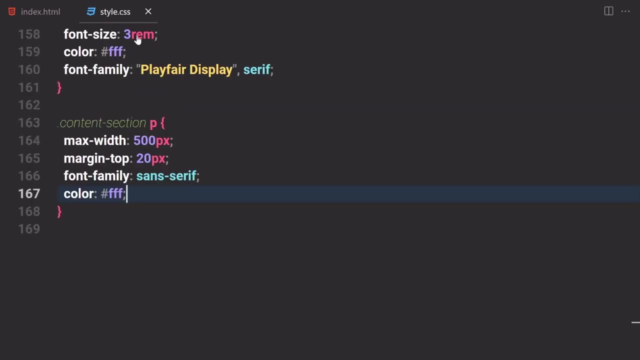 and, by the way, you can also change these text if you want to, but i'm not going to. so if you save that and we will see this card right here. but they aren't styled that much well, so we have provided a bit of coding for that, so we have to just first of all get this comment from here, and i'm going. 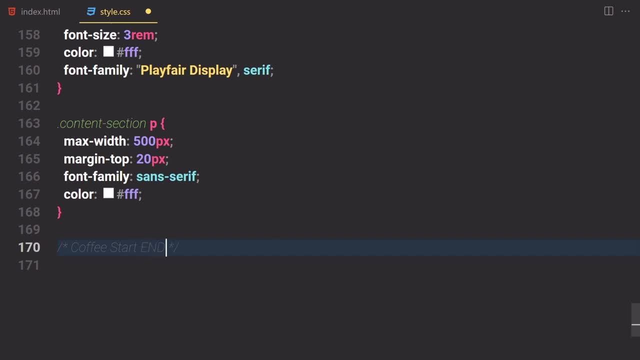 to put it right here and put at the end and the end. so i'm going to just zoom in a bit. first of all, now let's just start working on our product section. so i'm going to just select that product. oh my goodness, products section right here and margin will. margin of top will be just five frames. now let's just select our. 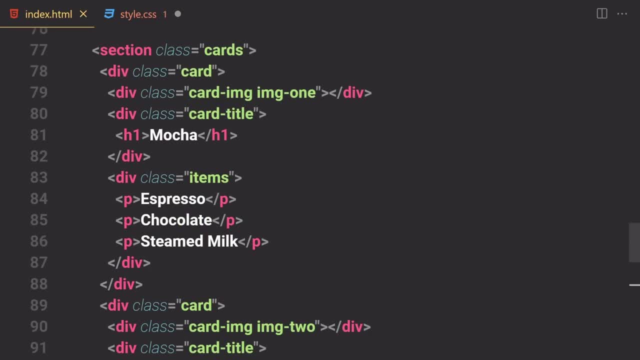 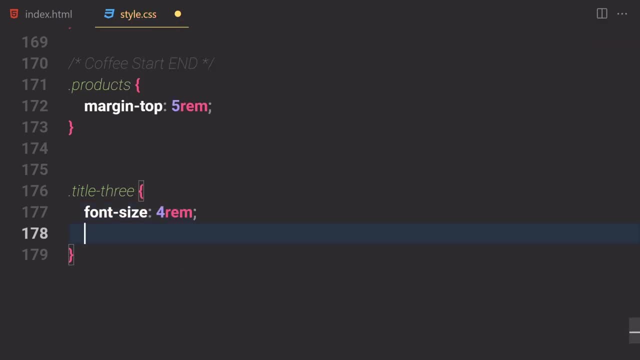 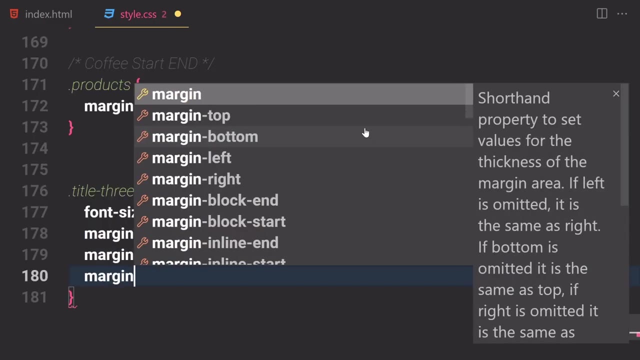 tile three in this case, because we provide this specifically, title three, right here. all right, so now let's just style that. so font size will be just four rim and margin to the left will be 10 rim and margin to the top will be also 10 rim and margin to the bottom. we could have also used 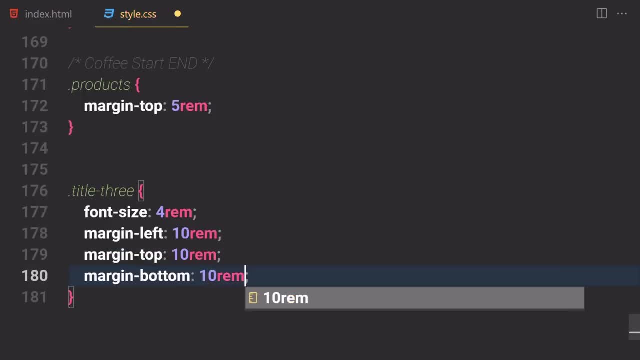 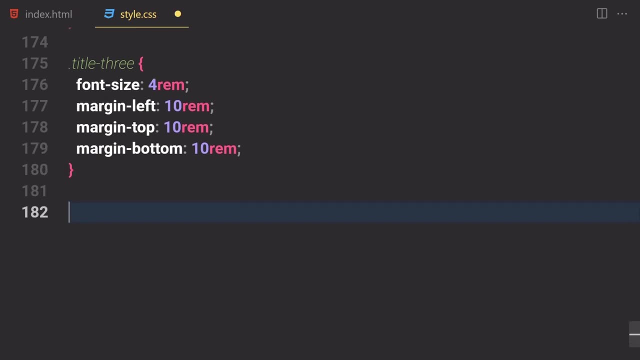 we should have used that shorthand, but anyways it will, it will do the work. so if you save that, and this is going to be it for our product section right here, so now, what else do we have to do now? let's just start working on our card section- a plural card section, not a. 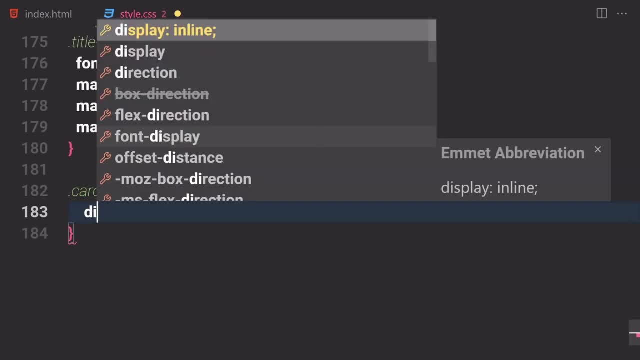 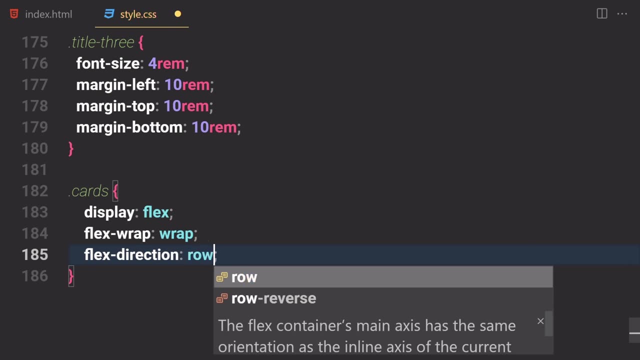 singular. so you're going to be selecting our card section and the display will be now set to totally flex. flex ramp will be now set to ramp. flex direction will be set to row, in this case, not column, and justify content will be space around and final property i'm going to use for a line. 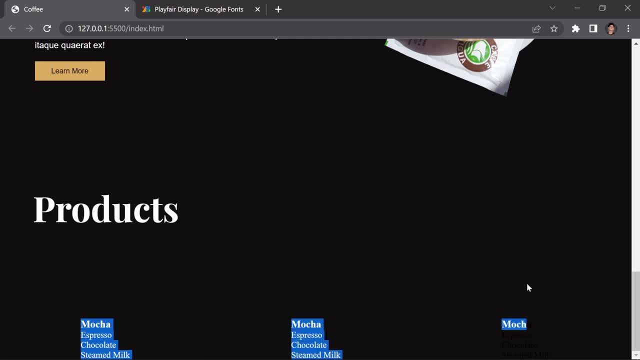 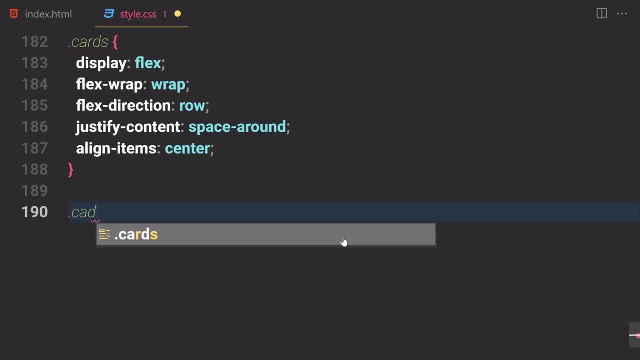 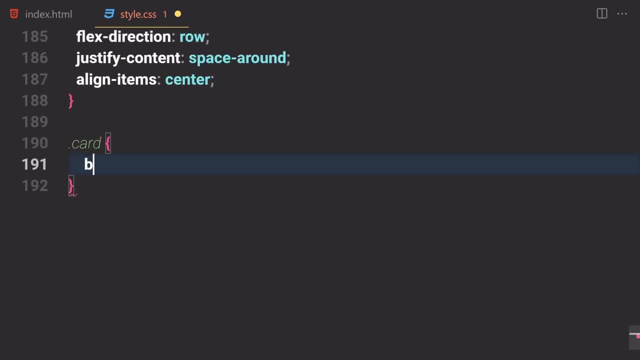 items of center and if you sell that. so here you can see, you're now getting, uh, our cards right here, but they aren't styled well. so now let's just style that a bit. so what do we have to do? we are going to be selecting order card, in this case, not cards, but just a singular card right here. all right, so now. 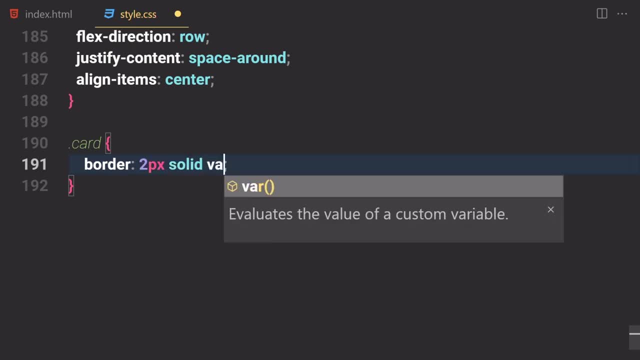 i'm going to just do, i'm going to provide a border of like two pixel solid and that kind of our main color, and if you sell that, yep, that's cool. uh, i guess that's that's cool. you know, i'm going to remove that, i'm going to change it to some. 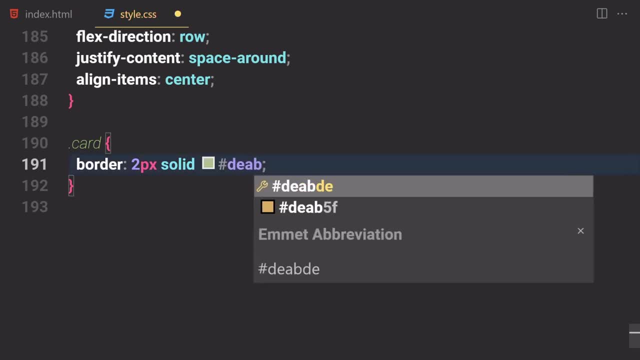 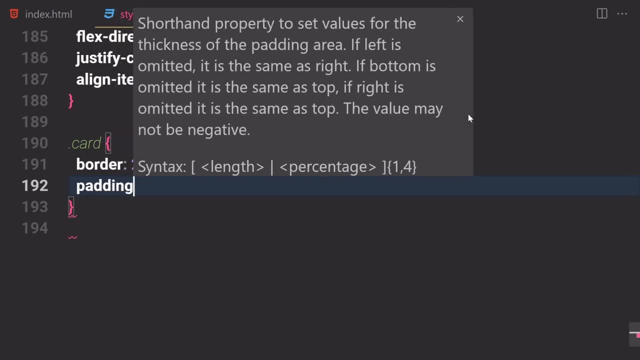 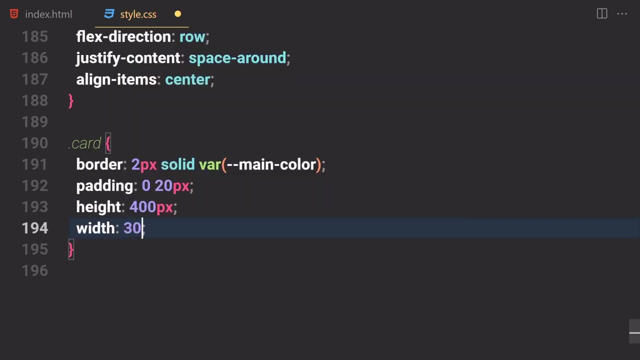 let me just write like d, e, a, b. okay, so that's the same color. i'm going to just change that to our main uh color right there anyway. so we can just provide a padding of zero for the top and bottom and 20 pixel for the left and right. height will be totally 400 pixel, the width will be just a 300. 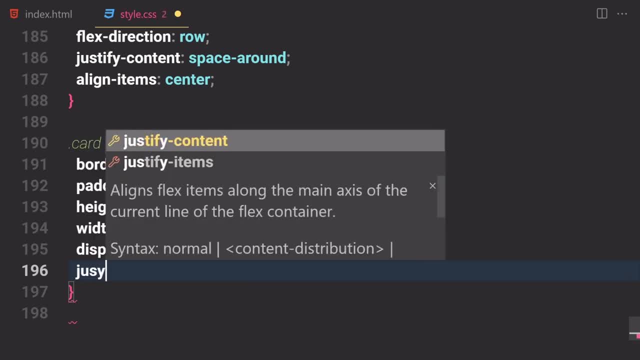 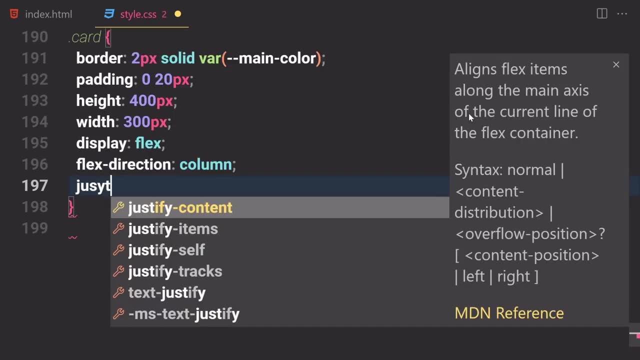 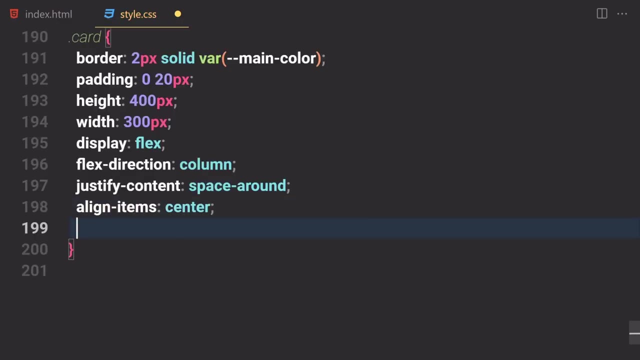 pixel and display will be totally flex. justify content will be column, not justify content. flex direction will be calling in this case. and now let's just use our justify content of space around, and now let's just use our align items of center and border radius will be now set. 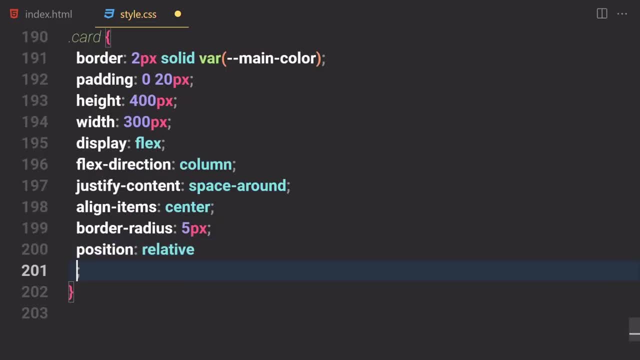 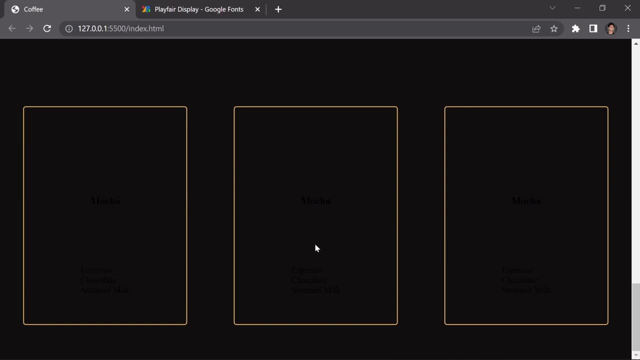 to 5 pixel and position we are going to be applying for it, so like relative positioning, and then let's just use our margin bottom of 4 ram. so now, if you save that, and this is how currently things looks like, but now let's just style or card title and card info or paragraphs, whatever you want to call. 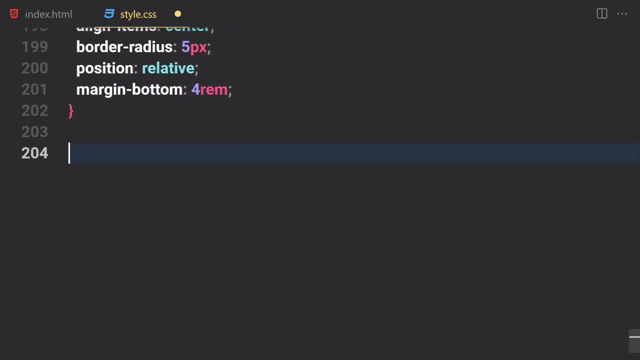 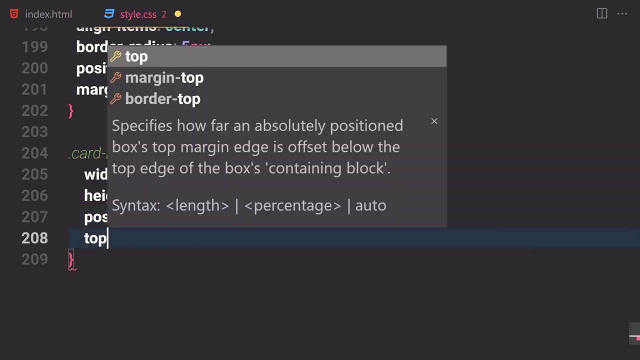 that. so now we are totally done with our card section. so now let's just use our card image. first we have to specify image for our cards, so to do that, we are going to be writing a width of 100 pixel and height will be also 100 pixel. let's just use a position of absolute on it and the 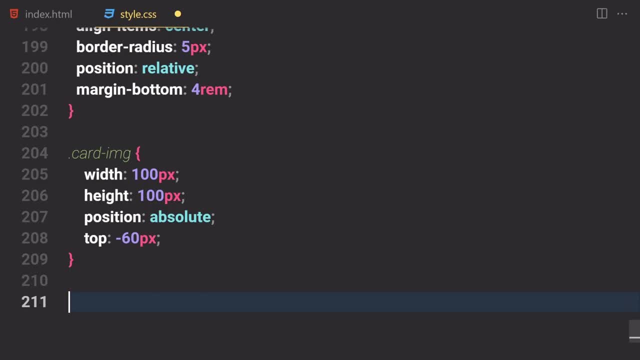 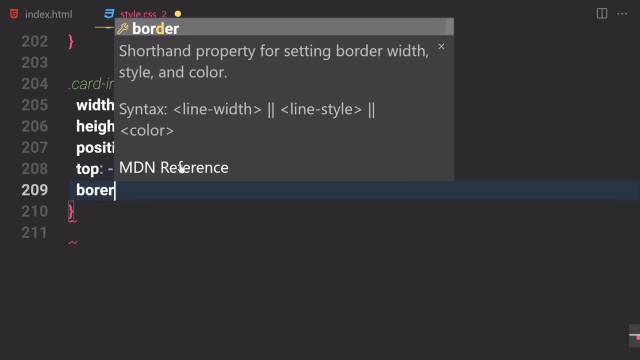 top value will be like 60 pixel in this case. and now let's just start working on our different kind of images. but before we do, first of all, let me just show you how it will look like. so i'm going to just write a border of two pixels solid and that a war of main colors, if you save that, and 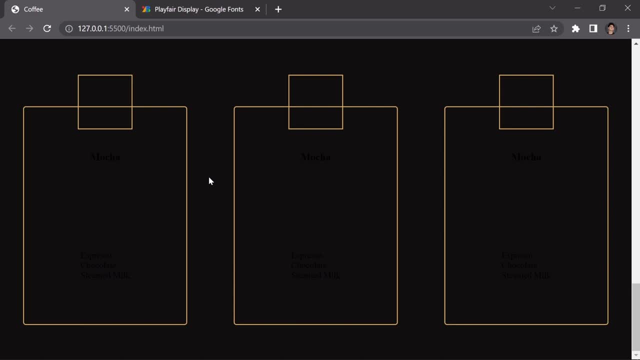 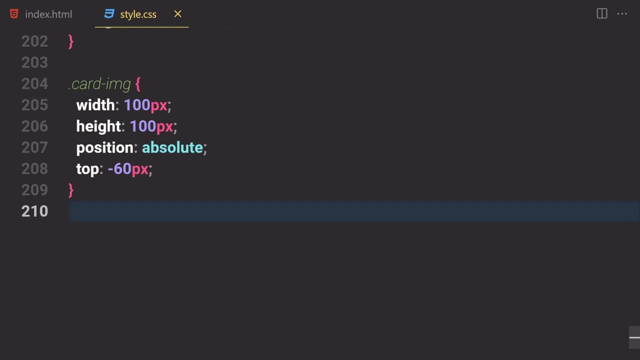 this is how it will looks like by default, so we can style that manually if you want to. so you know what i'm going to remove them. and now let's just start working on over different kind of images. so for this first card, we provide a class of img1 like image1. this is going to be our image 2. 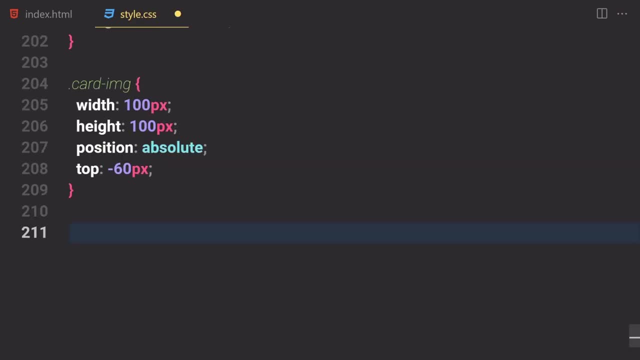 and i guess that will be it. okay. so now let's just select or image one. so i'm going to just write like img and 1.. now let's just use a background color of url in here. so i'm going to just put a url go to the images and i'm going to just put a background color of image1 and i'm going to just 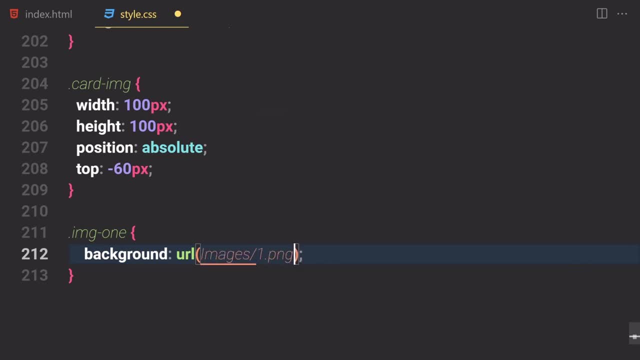 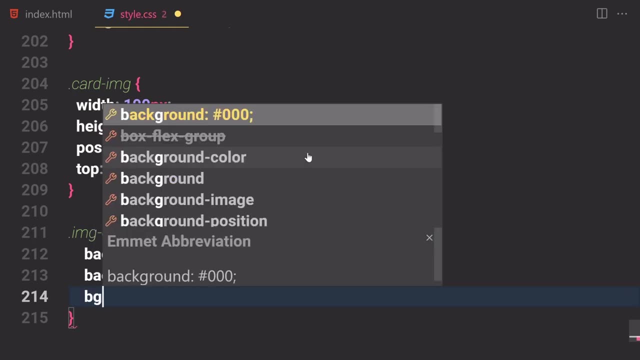 So now let's just use a background color of url in here. so i'm going to just put a url, go to the images section- i mean like images folder- and select our first image. so what else do we have to do? we have to use a background positioning of center, and now let's just use a background size of totally. 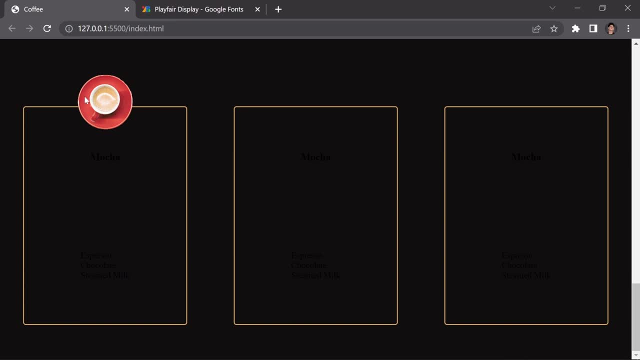 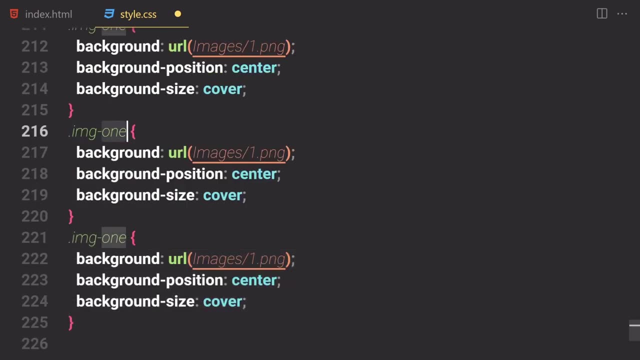 cover. so if you save that and here you can see, we have our first kind of image right here. so now let's just duplicate this code two times. so this first and this is the second one. so we have our image two. select our image two and this is going to be fine. so then we have our image three and 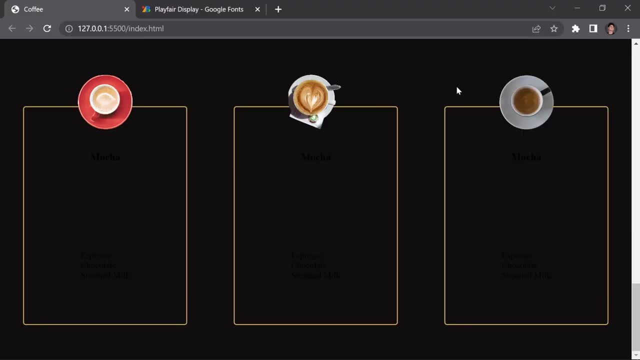 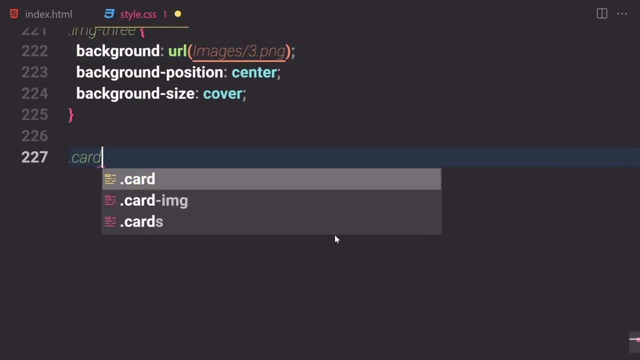 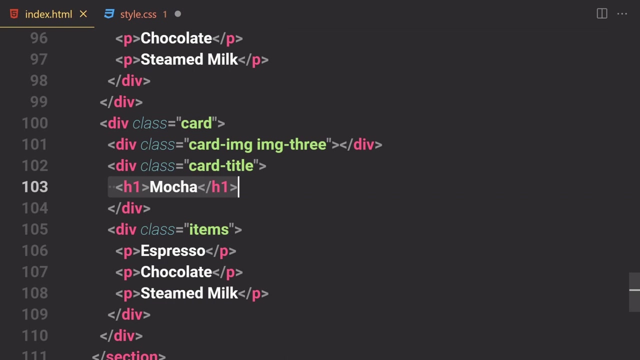 now let's just select our image three and now, if you save that, so we have all of these images right here, okay, so now let's just style these titles and stuff. so first of all, we are going to be using a card dash title. so which is that card? uh, title? right here, this one. so we are not going to be 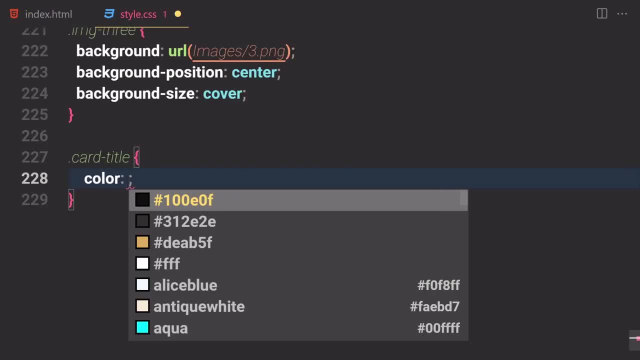 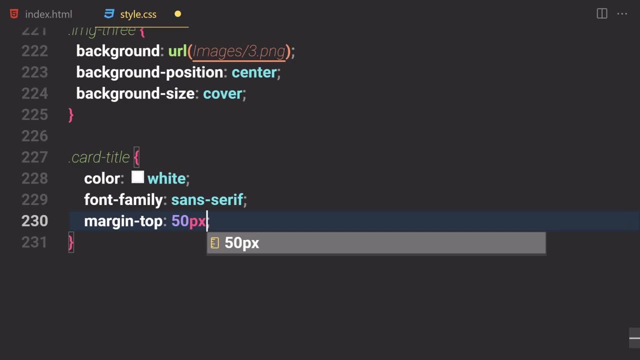 styling this one. so what do we have to do for that? we are going to be using a color of totally white, and now let's just use a font family of sans serif, in this case, and the margin top i'm going to give like 50 pixel. and now, if you save that, 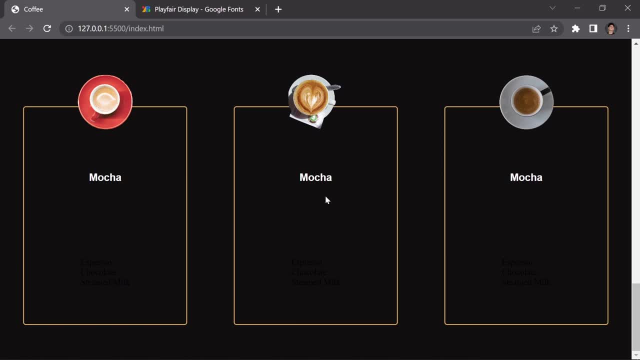 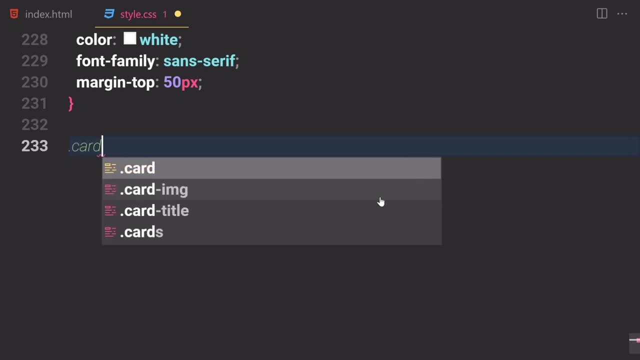 and boom, and this is how everything looks like, and you can just change these name if you want to. and now, what else do we have to do? we have to also style these paragraphs real quick, so we can just select our card and then items inside that card. and now let's just select our. 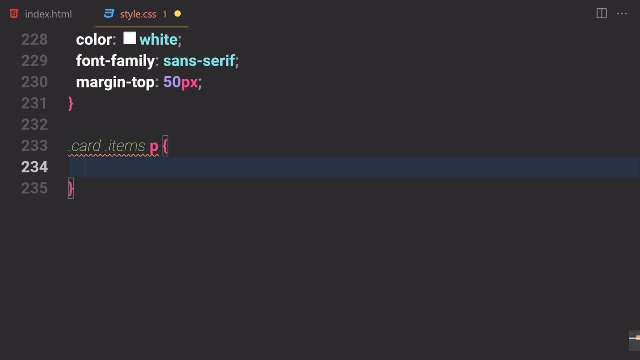 paragraph i, t e m s? yep, correct. so now let's just change the color to be totally white. margin for the top and bottom we have is a 20 pixel. for the left and right we have a zero pixel. font family will be totally sans serif, and if you save that- and this is how- 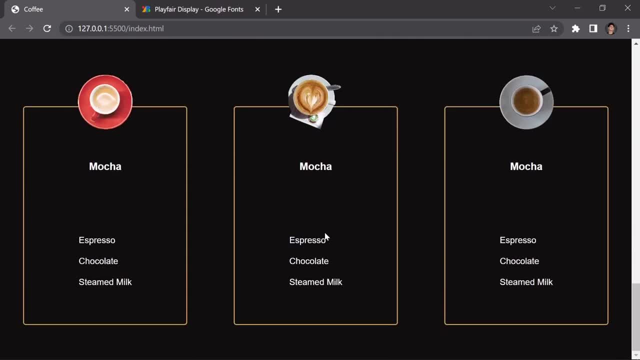 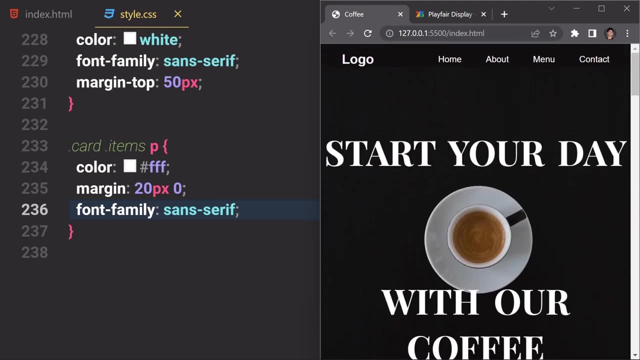 our card section looks like okay. so if you just make our screen size a bit smaller, it will just push it to a new line and this is how everything looks like for now. i know it's not responsive- we are- we are going to make that responsive just in a second, but for now everything looks cool. 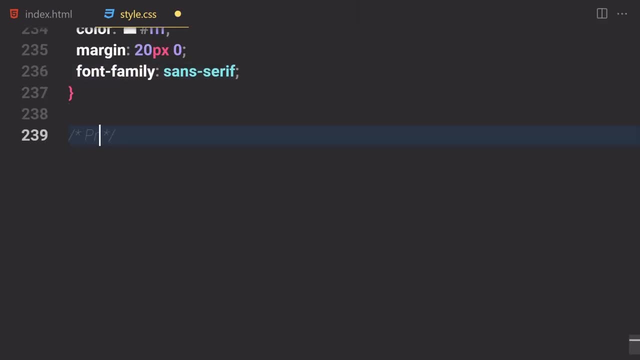 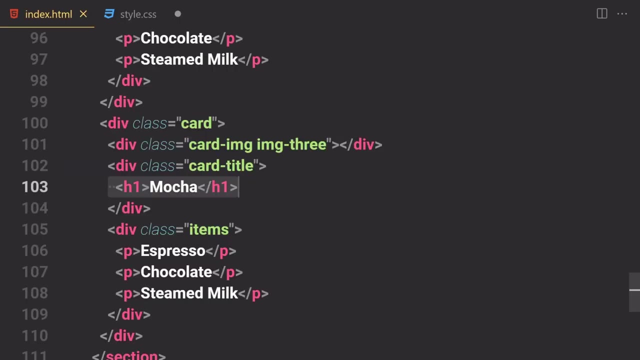 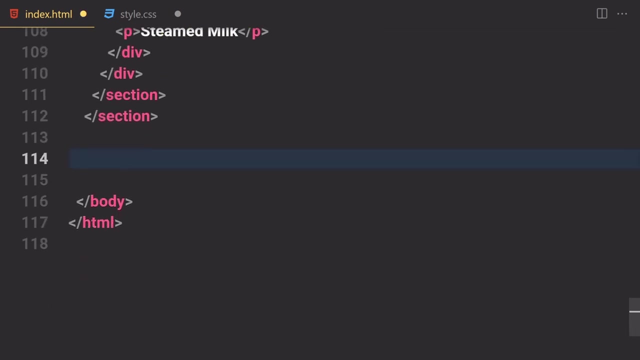 all right, so here we have to just write or uh products, products, uh section, and or i'm going to just put an in there. okay, so now let's just start working on our photo area, and that's going to be it for this project. all right, so outside from this section, we are going to be using first of all: 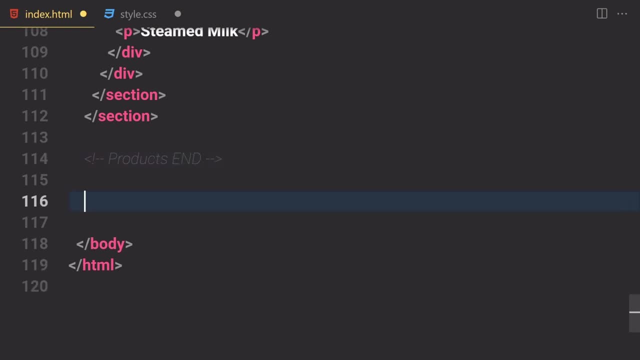 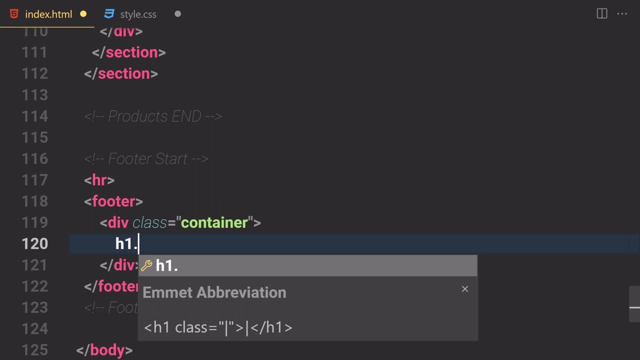 you know, i'm going to just write a products end and now let's just use or folder start and folder end. so we are going to be using hr for horizontal line and now let's just use our footer and inside this folder we are going to be writing our container. inside this container we are going to 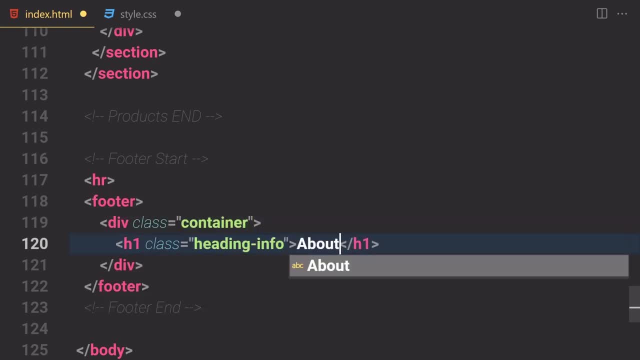 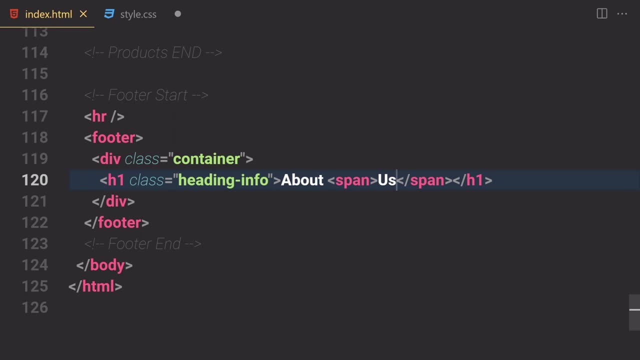 be using our heading info first of all, so we are going to be writing our about right here, and then we are going to be using a span of us, okay, so, if you save that, so this is how it looks like, and underneath this h1 we are going to be writing a paragraph with a lot of lorem ipsum inside there. 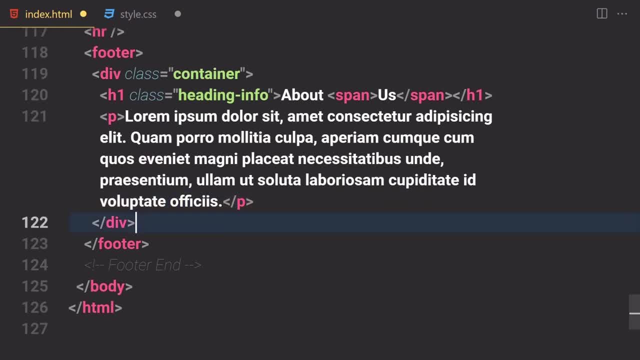 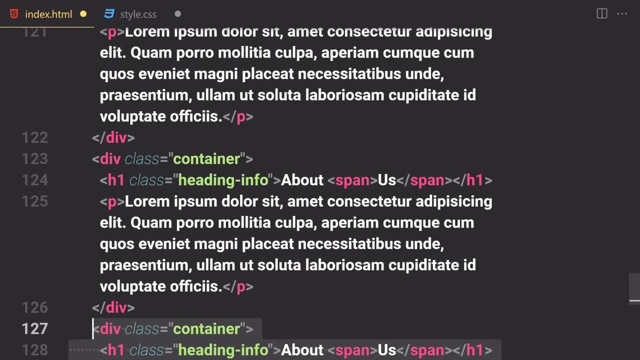 and i guess that would be fine. and now, underneath this div, uh, what else do you have to do? underneath this div? we have to. you know, i'm going to duplicate that a few times. why not? or can't i? you know what? let's just see, i'm going to duplicate this two times. so one, two. so we have. 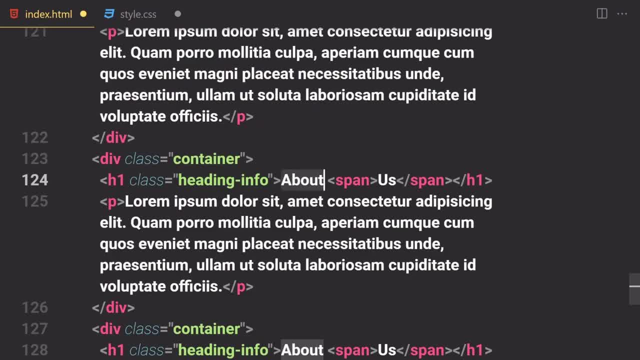 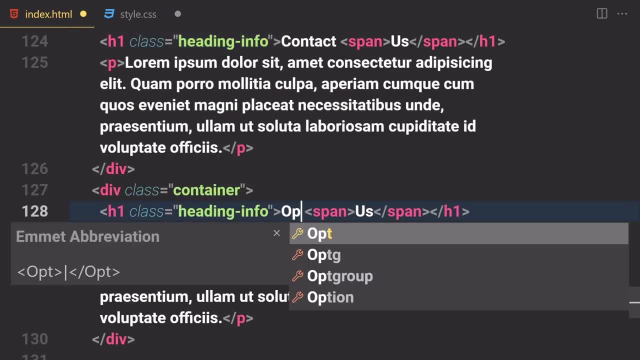 selected prepcweb. we are going to make a list of all the projects that we are. i suppose we may like click on these as its tab. ok, so completely dropdown. and here you can see the page is complete, providing info. it is now adding info. now let's just change the title to be like: 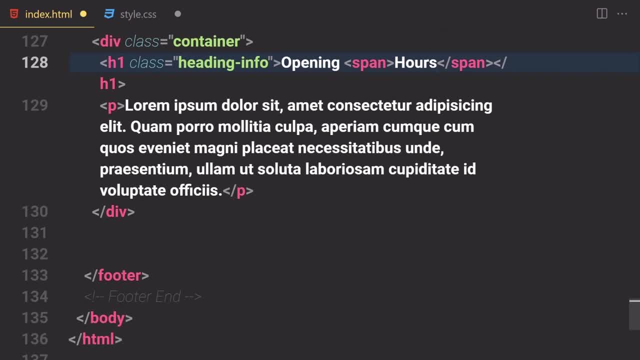 something else, maybe contact in this case. so contact us, uh, about us, and opening howards would be fine. so o-p-e-n-i-n-g and then cards. okay, so we are now totally done with this container section. then, outside from this div, what else do you have to do? we are going to be writing um. 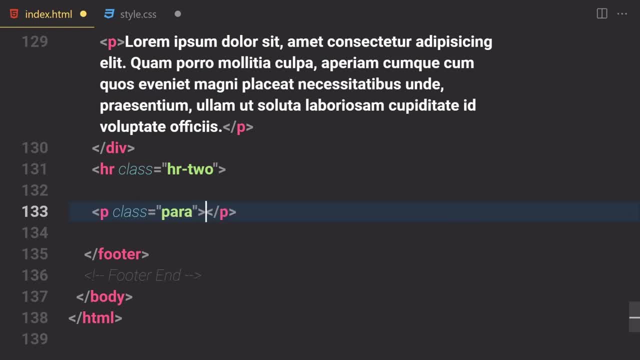 So I'm going to just write a paragraph with a class of para or credit. wouldn't it be fine if you just write a class of credit? you know I'm going to go with a para class. I'm going to just sort of like a copy right and then add similar 2023. In this case, of Hussein web dev. you can. 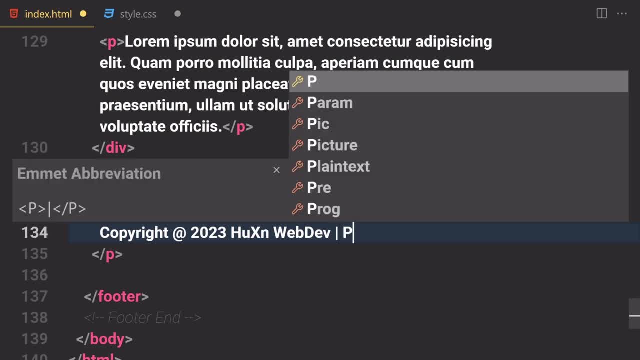 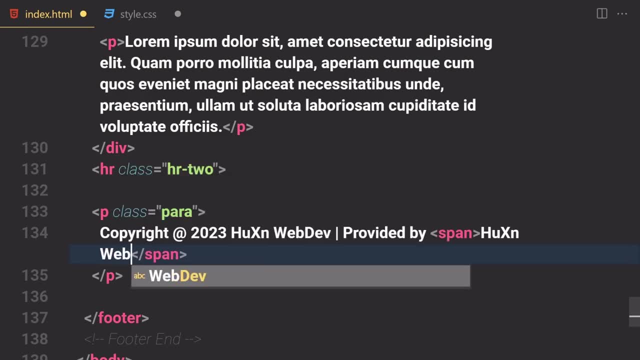 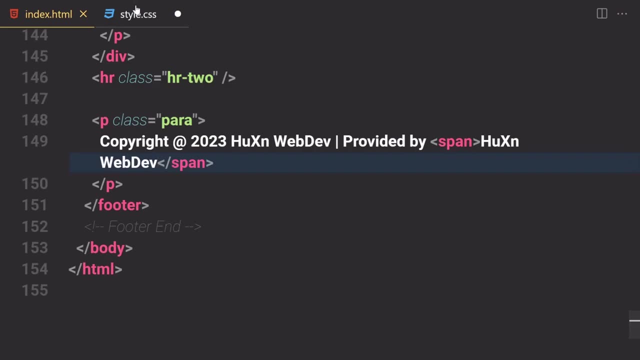 write your own name if you want to, because this project is now totally yours. What will I do with this? friend? projects are provided by span of Hussein web dev. So if you sell a file and this is how it looks like right now, I'm going to jump into my style sheet right now. And now, let's just 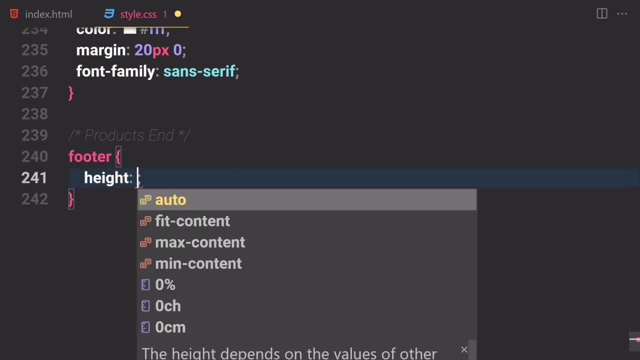 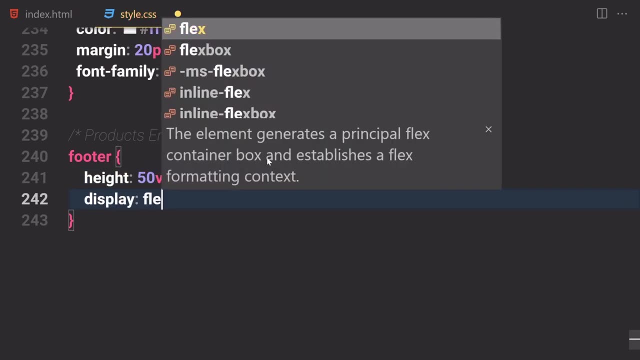 tie it up there. So first of all we are going to be styling or further area. I'm going to give him a height of like 500, not 550 VH, and display will be totally flex and flex wrap will be set to wrap a line. 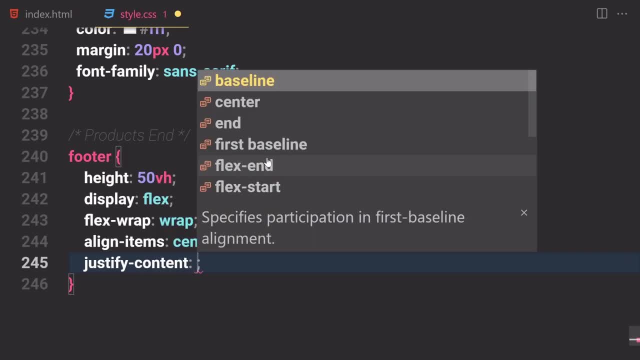 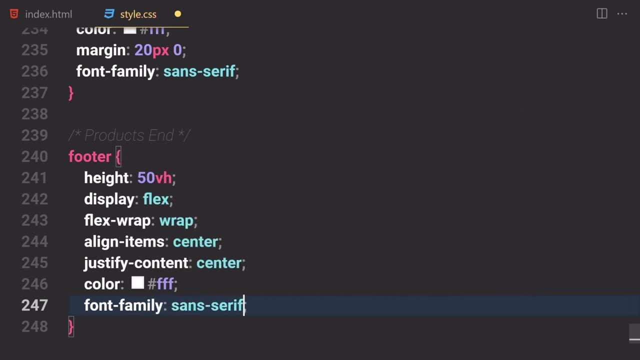 Items will be now set to totally center. justify content will be now set to totally center. color will be totally set to white. And for family I'm going to set that like sans serif in this case. So if you sell that and boom, everything is now magically in here. So now let's just take care. 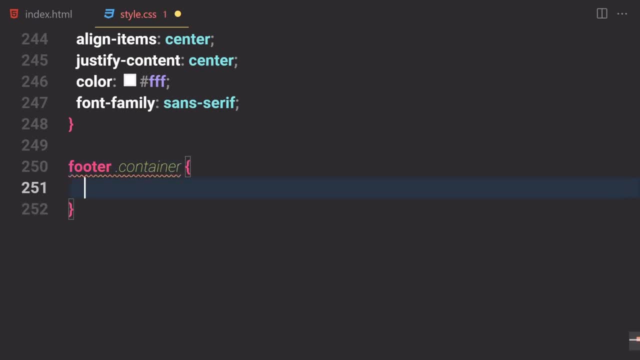 of their alignments. we are going to be selecting our footer And then let's just select our container inside that footer. we are going to be providing a margin of 20 pixel. the max width I'm going to provide is like 300 pixels, And also the text alignment will be set to now set to center. 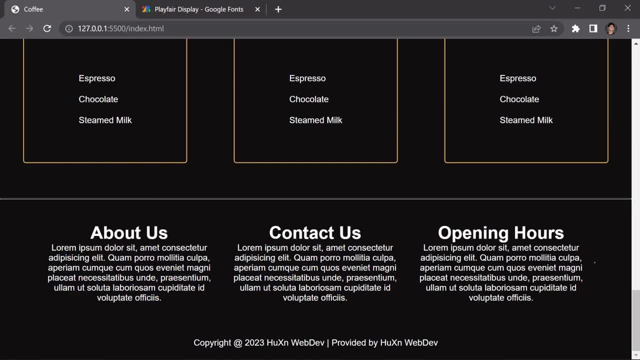 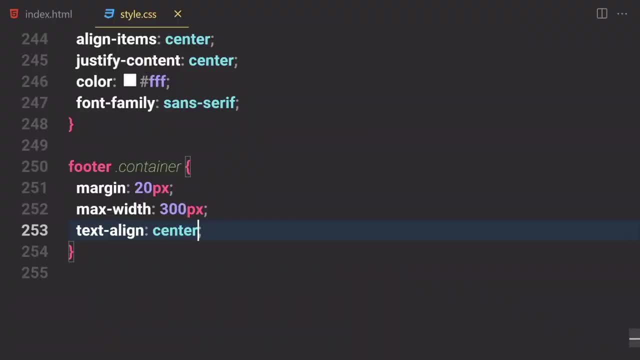 So if you sell that and this is how currently things looks like right now, Alright, so it's looking awful, I know that. But what else can we do? we can just improve that heading info clause, which is provided. So you're going to be selecting this footer and then heading and then info. So 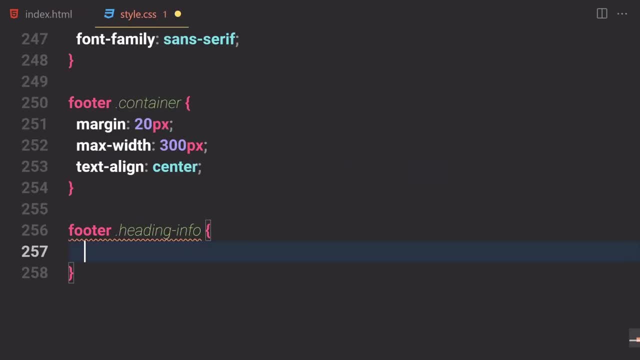 let's just select this header and then heading info real quick And let's just provide a margin of bottom of 20 pixel. In this case, just one x would be fine. And finally, let's just select our footer and paragraph, And we are going to be using a line height of 25 pixel in this case. 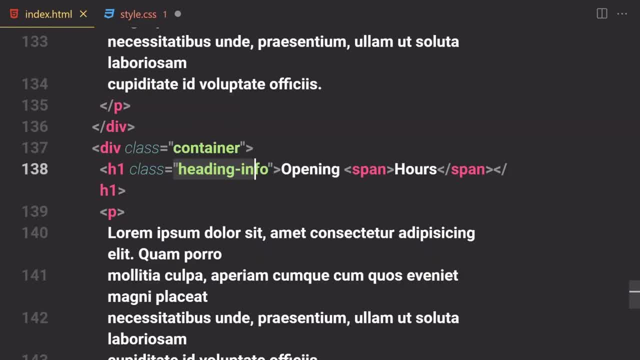 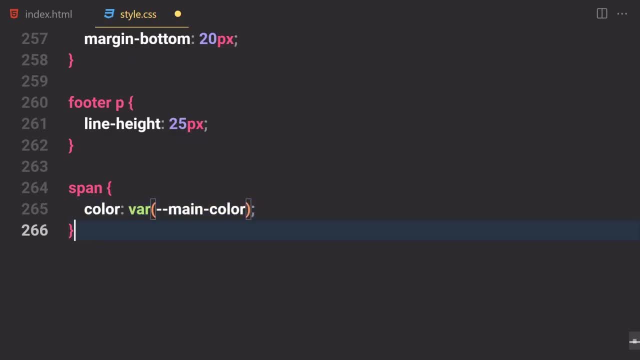 and also select or span, which we provide for a new color, which is this color right here. So we are going to be game a class of not a class, but a color, of their main color And, finally, you know, I'm going to save this file. So this is how currently things looks like And I know this. 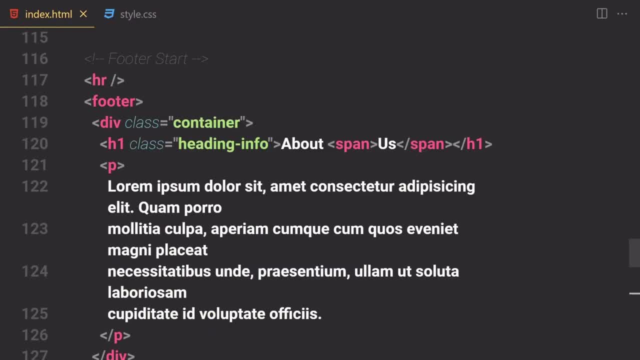 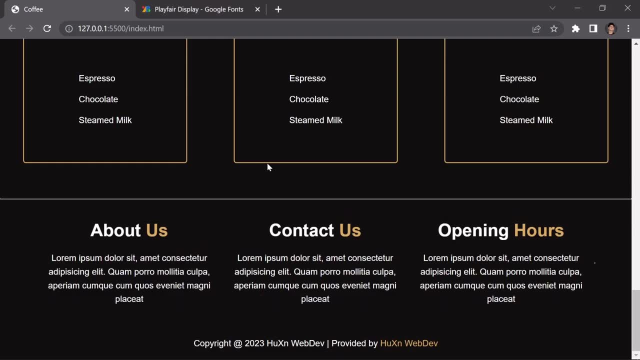 is a lot of text, So we have to just delete a few of them. So I want to select this portion and hit delete And bye, bye And so, and this how things looks like. I know it's a lot, You know what. 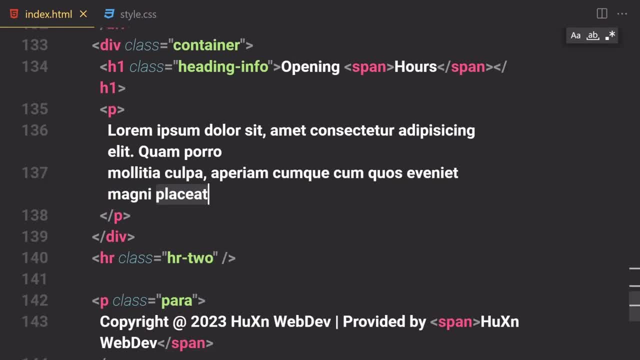 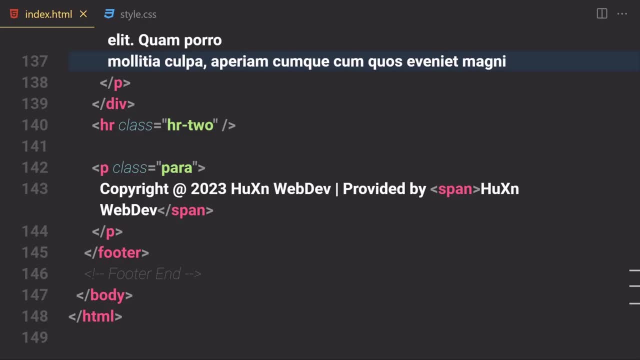 I'm going to select that place placenta, And let's just remove that and save it. Yep, that's cool Anyways. so let's just take care of their horizontal line, which we provide right here. So we have HR here and then we have their HR to right here. So now let's just take care of. 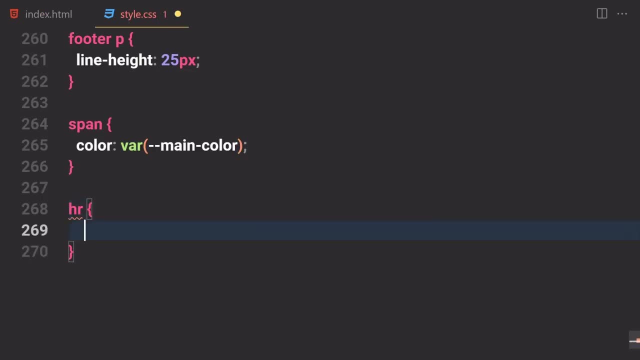 that real quick. So we are going to be using HR And let's just write a margin bottom for it like 20 pixel, And border color I'm going to provide is their totally main color, which we just provide, And then width will be 500 pixel And I want to give a margin of zero. 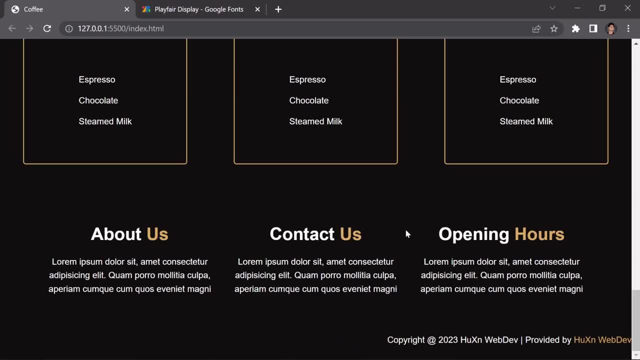 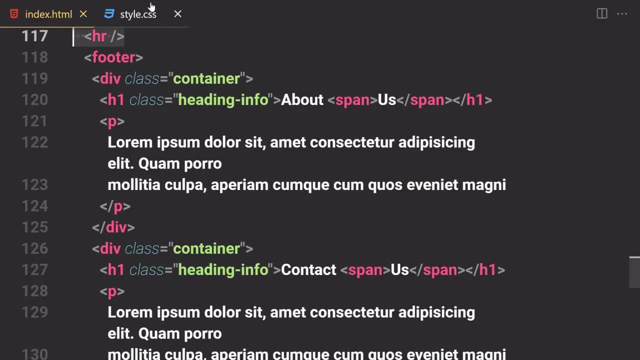 auto. So it will be now totally at the center. Okay, so what's wrong? Oh my god, Something wrong. So it's now taking this area. you know, I'm going to sell that a bit just in a second, So let's just. 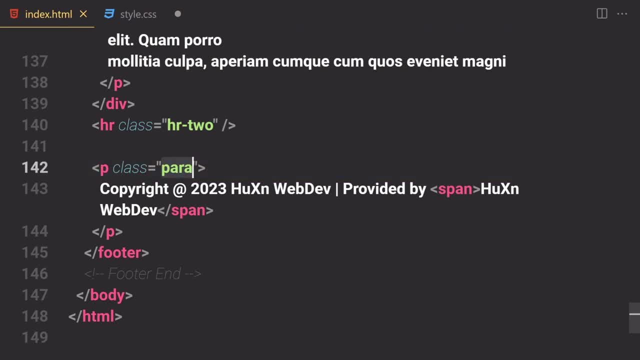 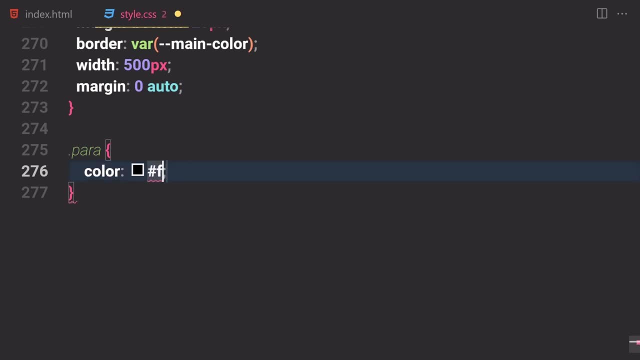 select their para, which is their para clause. And now let's just take care of their real quick. I'm going to select their para clause. the color- I'm going to just write a color will be totally white And the font family I'm going to set that to like. sans serif text align will be now set to. 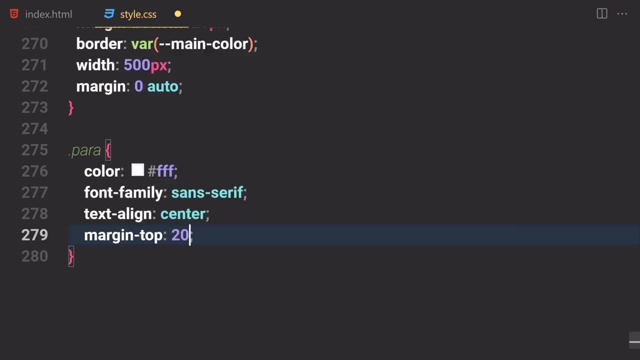 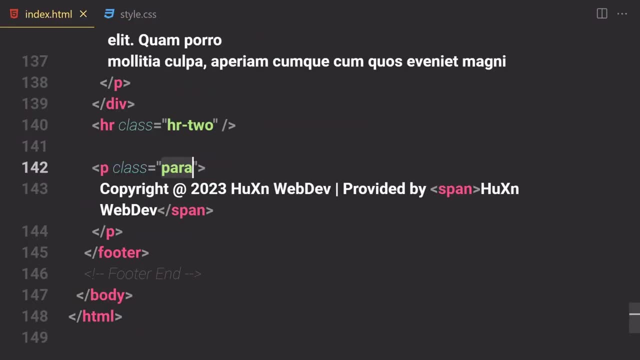 center and margin At the top. I'm going to just give him like 20 pixel and knife. you sell that. Yeah, this is looking cool, But I don't know what's happening to that HRs. We have HR one and then we have HR two, But I don't know what's happening to the HRs. It's looking awful. 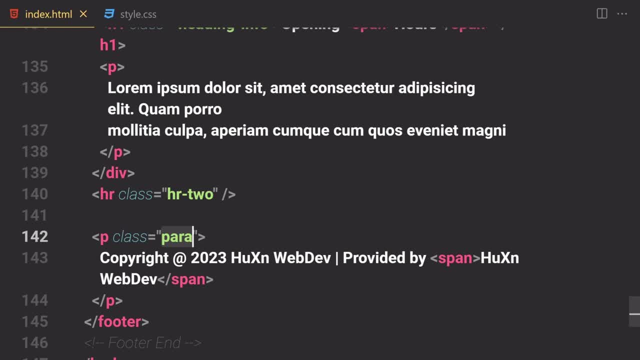 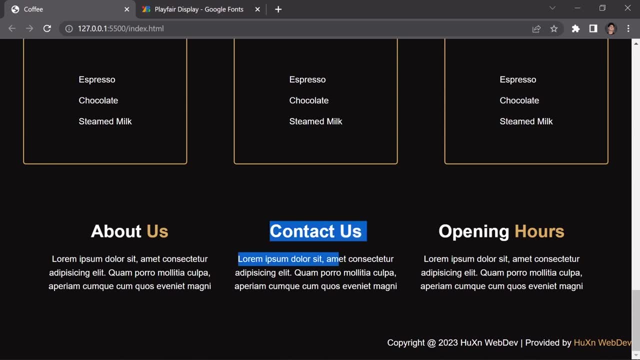 Well, what if I just remove these HRs? You know what if I remove that? that would be cool. So we have a width of 500 pixel in there. we are not wrapping more text inside there, do we? You know, I'm going to remove this HR And I'm going to also remove this HR from there. 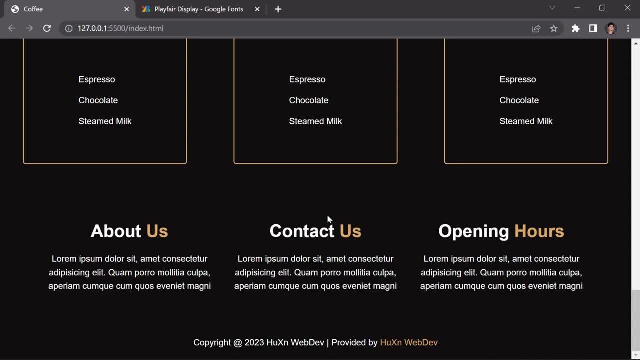 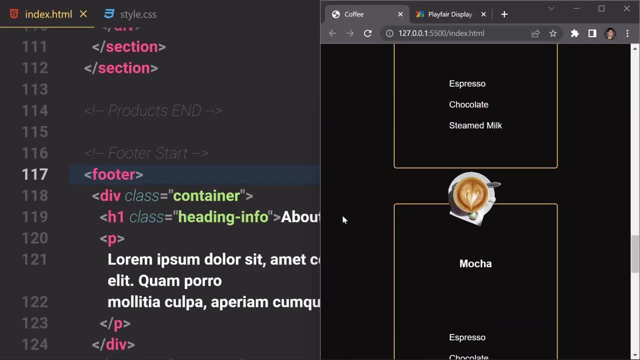 And yep, that's looking cool. If you want to pour a line, so you can. but I guess this UI is looking cool. But now we are totally done with our project. But here's the thing: it's not responsive. So for that we have fried a little bit of media queries. 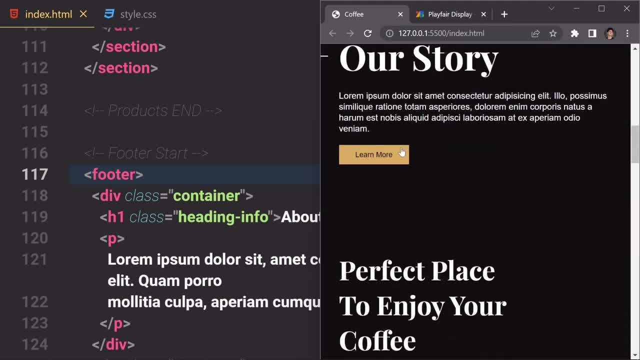 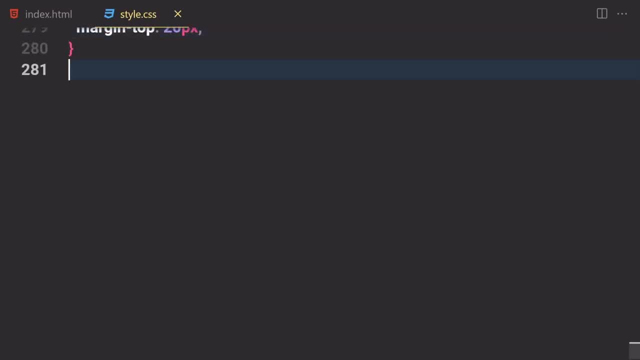 In here So you can see these texts is huge. This section is not looking better, And now let's just take care of that by using media queries. So I'm going to just write project N And now let's just write like risk pawn sale nurse. Okay, I guess I misspelled it. 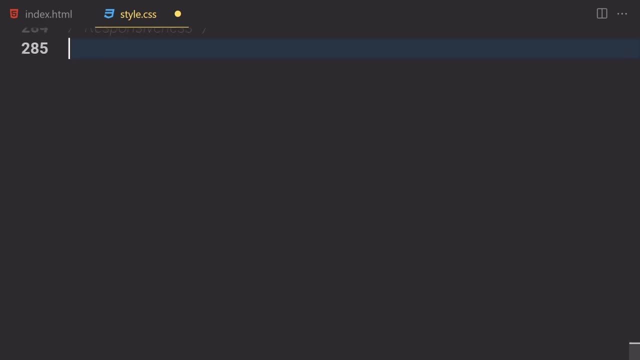 But you know what, who cares? You get the idea. So you're going to be using a media for only screen. Use your own webinars. PREEEEEEEEEEEEEEEEEEEEEEEEEEEEEEEEEEEEEEEEEEEEEEEEEEEEEEEEEEEEEEEEEEEEEEEEEEEEEEEEEEEEEEEEEEEEEEEEEEEEEEEEE. 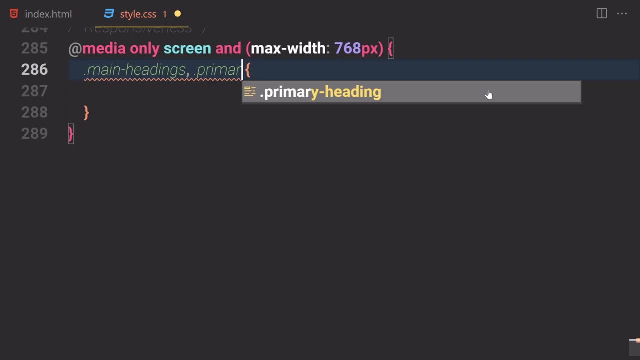 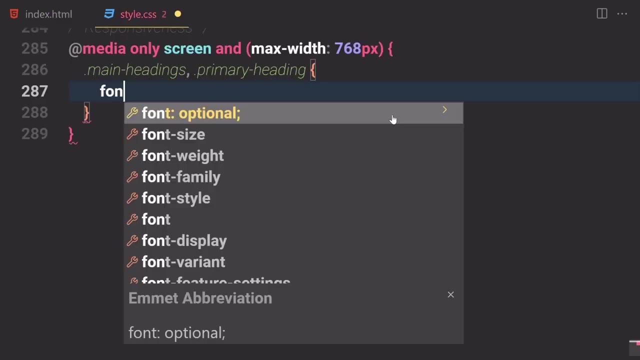 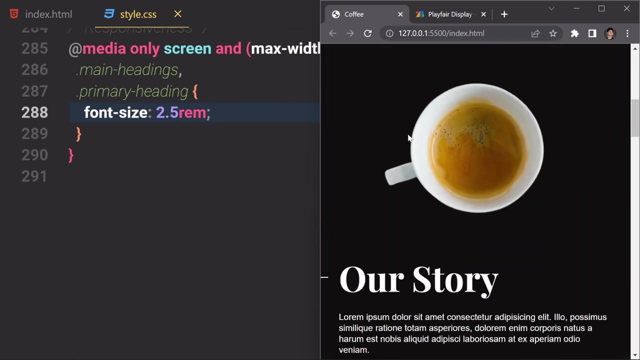 Come, so primary headings as well. is that a head? yeah, that was a heading. i'm totally sure it's a heading, not headings. all right, so now let's just use a font size of 2.5 rim and save that and boom, this is how it looks like right now. all right, so now let's just take care of this section area. so for there. 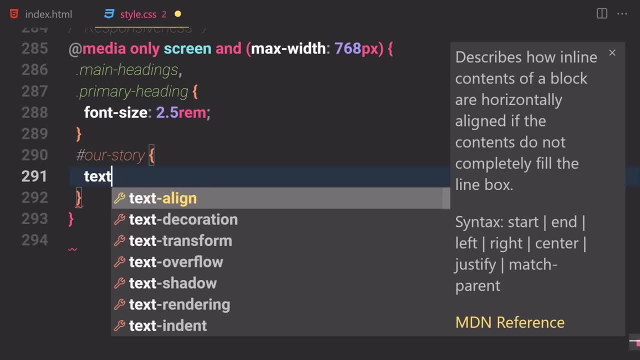 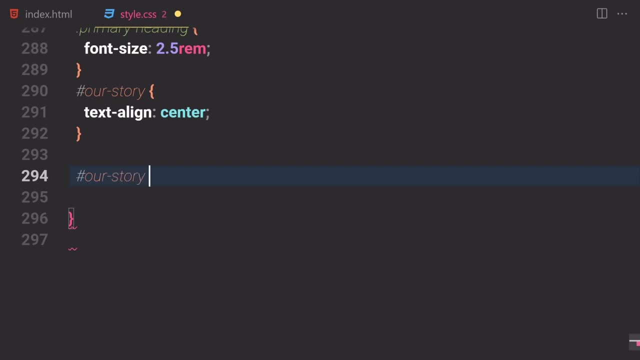 we have to select it by using or story, and now let's just use a text align of center and also take care of their title real quick. so i'm going to just select or story and then title of transform are translated to the x-axis of 50 pixel. so now i'm going to save that for now and this is how. 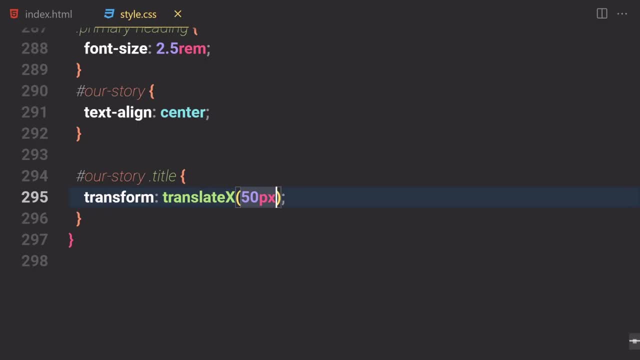 it looks like right now, and you know what. this line is not looking better. so i'm going to remove this line real quick. i'm going to write like or story and then let's select or line and write a display for that like none. so save it and yeah. 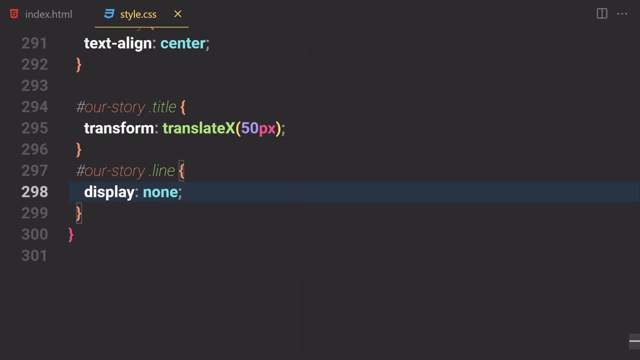 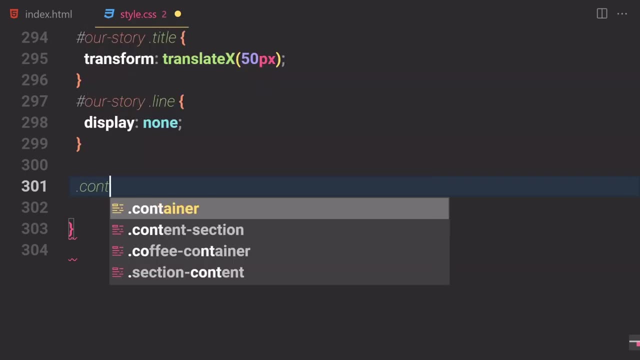 this is how it looks like right now, and then let's just use a text align of center, and also this is looking a bit better in the previous version anyway. so now let's just take care of that content section which we have right here. so now let's just take care of that. i'm going to just 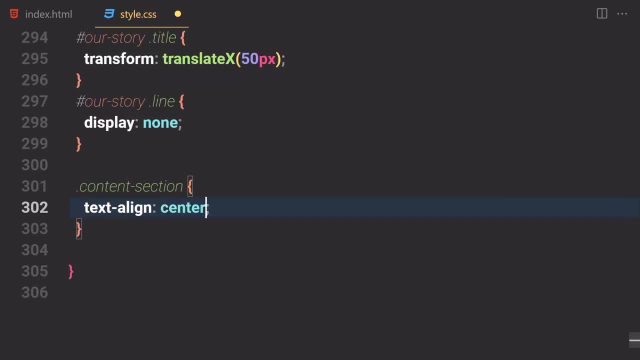 select my content section right here and text alignment. i'm going to just set everything to be centered. so if you save that, it's looking horrible. now let's just select or image section. so for that we are going to be first of all, you know what. first of all, let's just select or 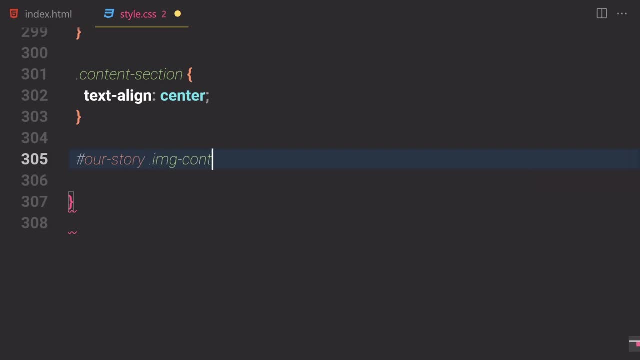 story, select or image container, container. and now let's just select our image inside there and i'm going to provide a width to be like 70 percent and i'm going to also provide a text alignment which will be now set to center. margin will be set to zero in auto and now let's just take care of that image container. so i'm 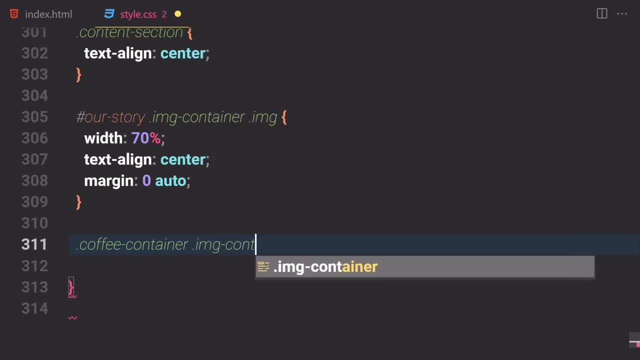 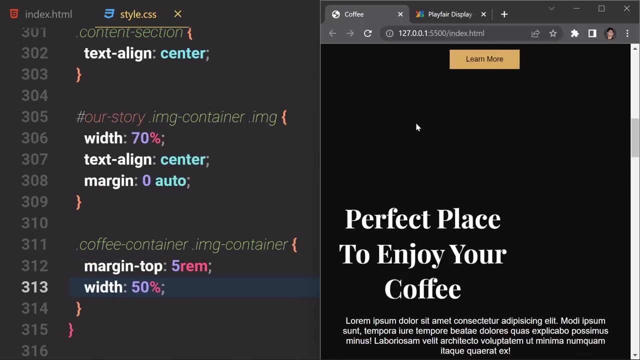 going to select a coffee container and write an image container right here and i'm going to put a margin of top of five frames and the width will be 50 percent. and now, if you save that, okay, so it's looking better. i don't know what's happening to this one. 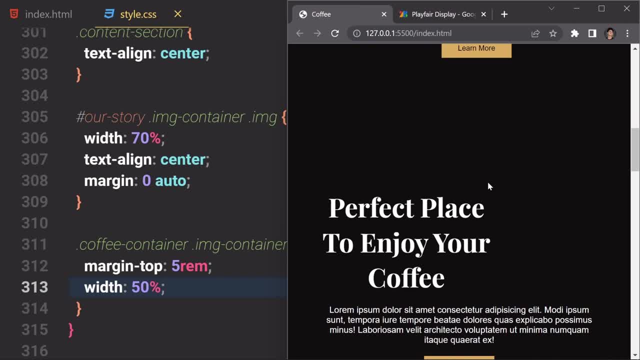 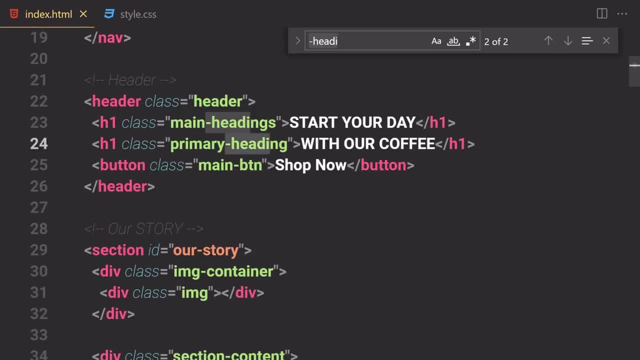 you know what. you can play around with that if you want to, but in my case i'm going to just make it so that we don't have any scroll bars and stuff. we can change this title. what is it on the class of this perfect place? uh, perfect place. so we have title two and if we select like, uh, i don't know is. 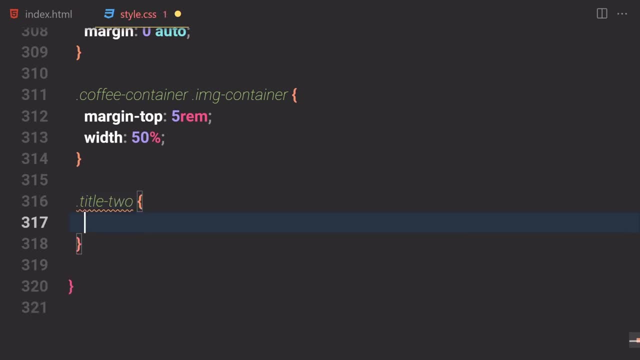 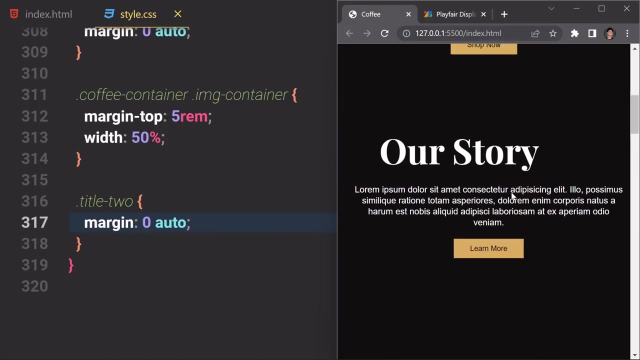 that a title two, title two of border: 10 pixels, solid red and if you save that, yep, that's it. use a margin of margin of zero. auto on it. all right, so it's not perfectly at the center. it's looking better right now, or story, uh, or 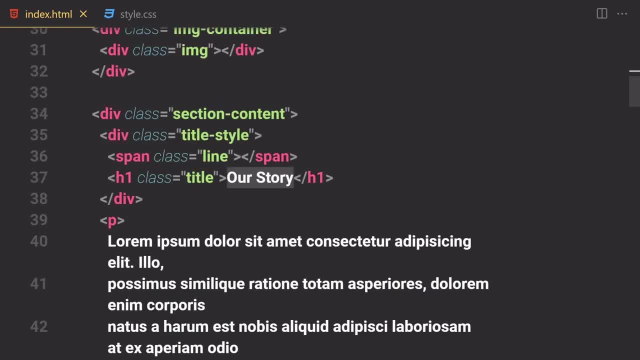 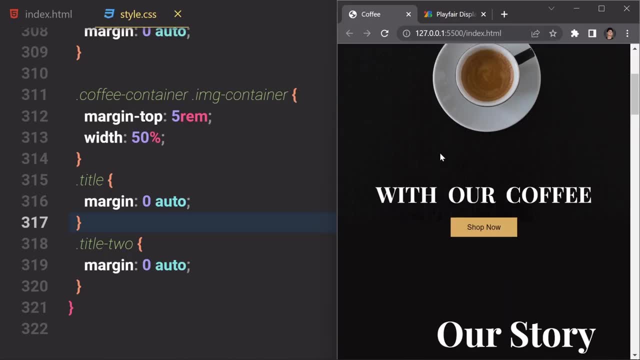 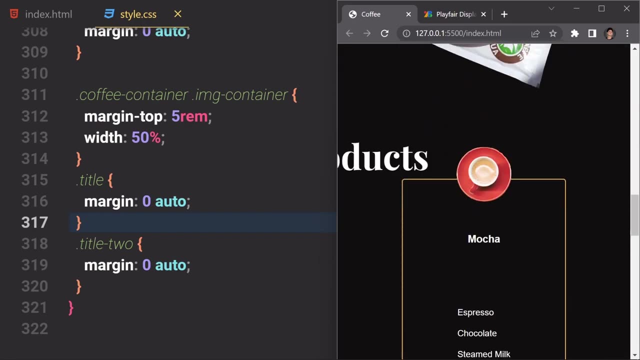 story, and now let's just select that real quick. that class is titled, so we are going to be using our title of margin zero auto in this case as well. so, yep, everything is better looking right now. then you can just tweak around it if you want to, but in my case, this is looking better. now let's. 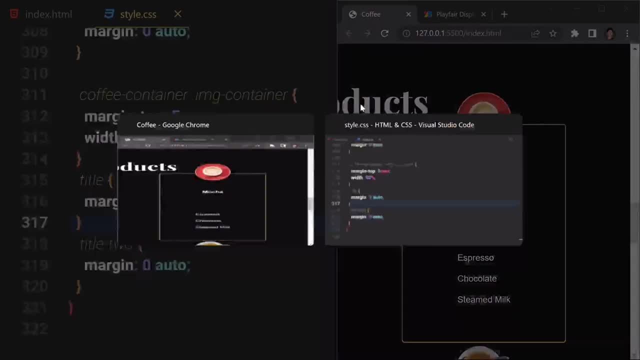 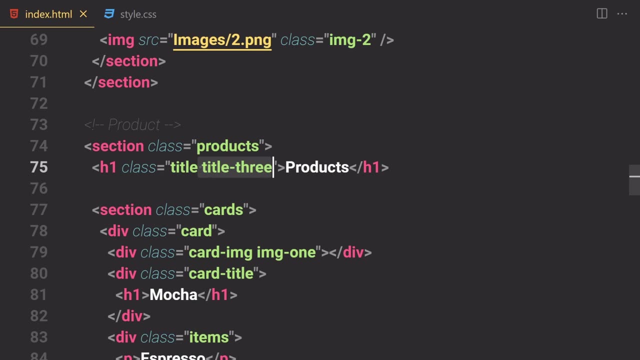 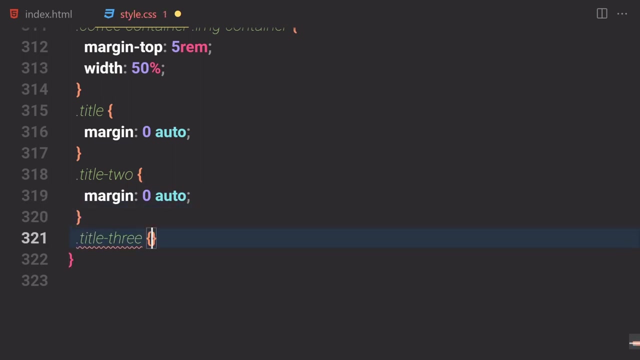 just take care of. uh, okay, so this is looking bad. now let's just select our product section. so we have title three for that, so we are going to be copying this one and let's just, uh, select that title three, like so i want to copy there real quick and i want to paste this margin zero, auto in there. so 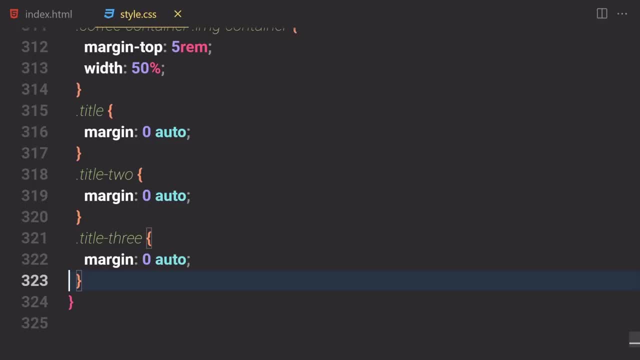 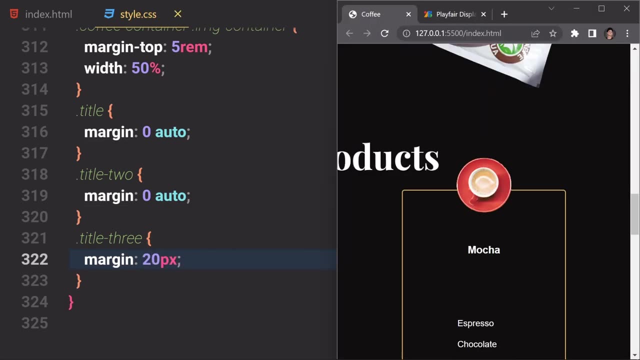 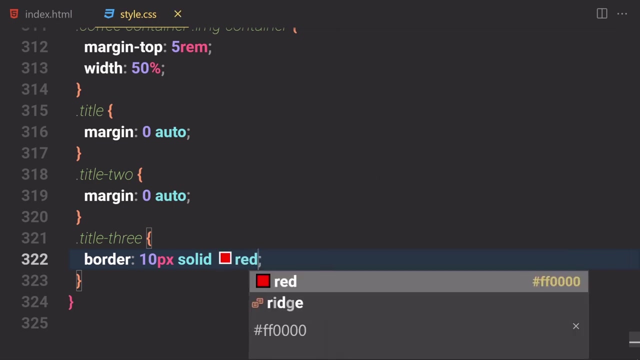 it's looking better, okay, so it's still looking awful. so you know what? i'm going to provide a margin for, uh, like maybe 20 pixel. so save that, okay. so it's not working. now i'm just i'm going to just write like a border of 10 pixel, solid red, right here. so if 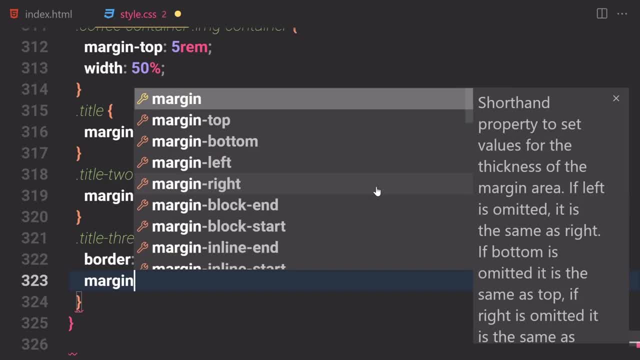 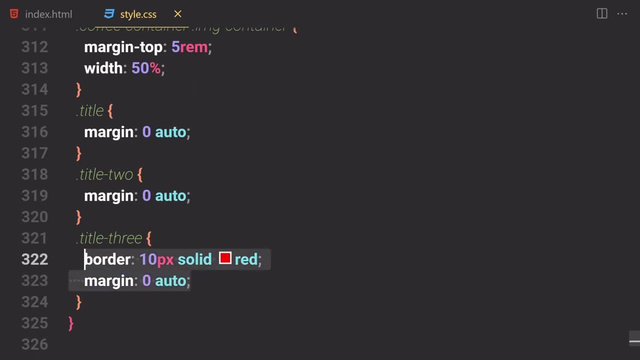 you save that certain value selected. so i'm going to just use like a margin of zero auto. and now if you sell there, it's not working, i don't know why. you know what. instead of doing all of that, i'm going to just use like a display of none. so if you save that, yep, that's looking better and we can. 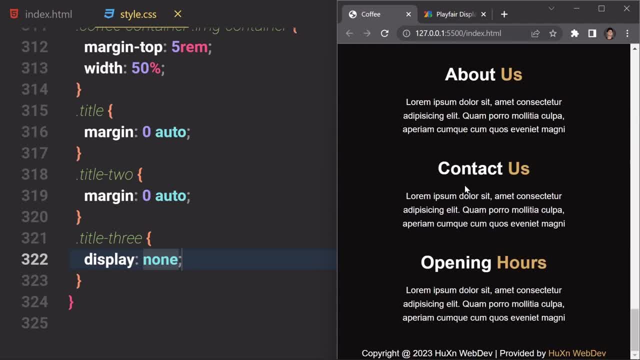 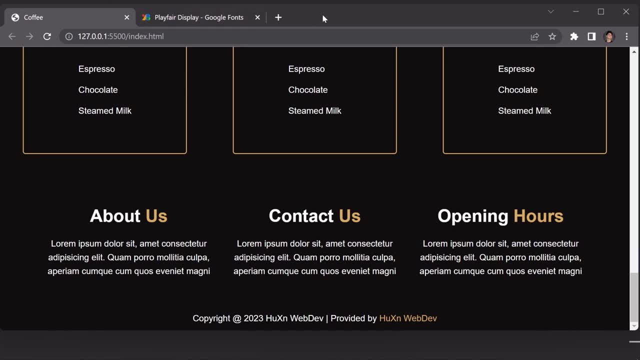 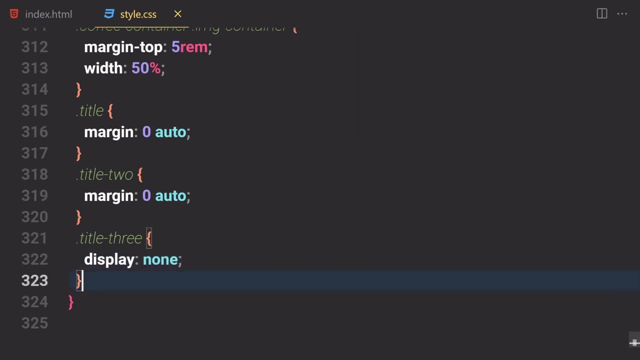 also provide uh spacing and stuff if you want to. but i guess everything is looking better right now, bit more smaller, and now let's just check him out- make it smaller so we do have that scrollbar right here. so now let's just take care of that para real quick. so what do we have to do? i'm going to 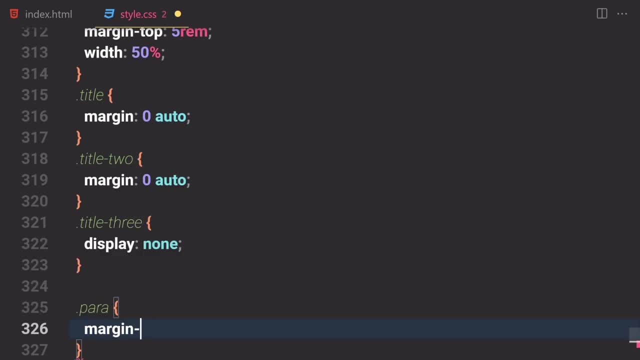 select my para and i'm going to provide a margin of a top of like 10 rem. so if you save that, it'll not push it to the bottom. uh, you don't want that. you don't want this to save it. you know i'm going. 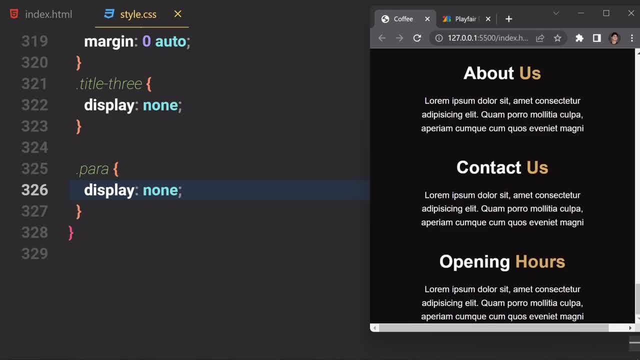 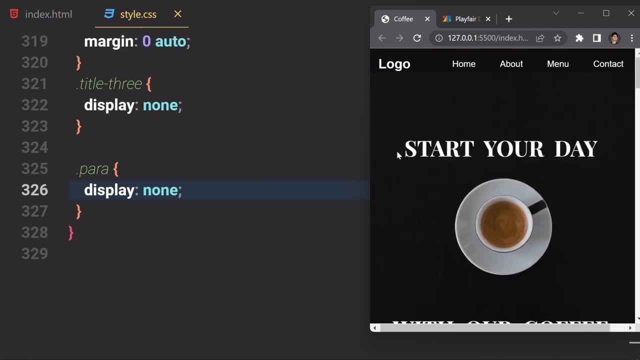 to also remove this para class as well, so the display will be none. so if you save that- and yeah, that's looking better, for now i know why we are getting this scrollbar from, but we are not totally done with this section. i'm going to make it bigger and yeah, congratulations, we. 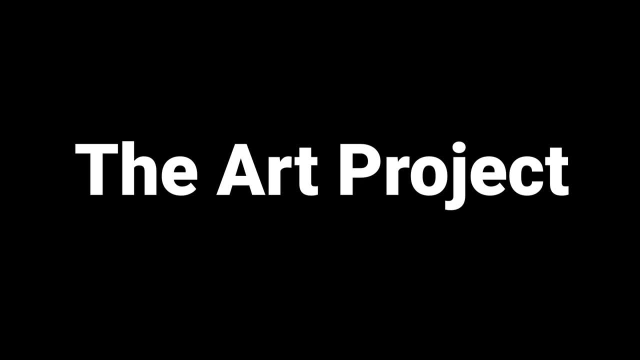 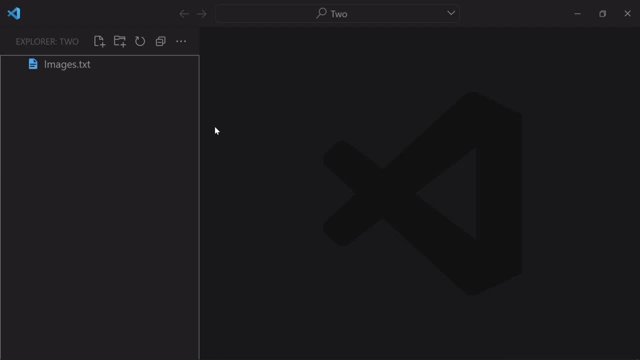 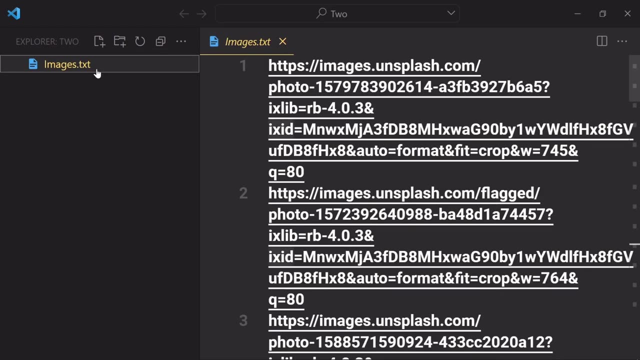 now successfully built our first project. all right, guys. so if you want to follow along with this video, first of all you will find a link in the description below which will bring you to my github repository, and in my github repository you will find this imagestxt file. these are nothing more, but all of the images which you are going to be using in this project. 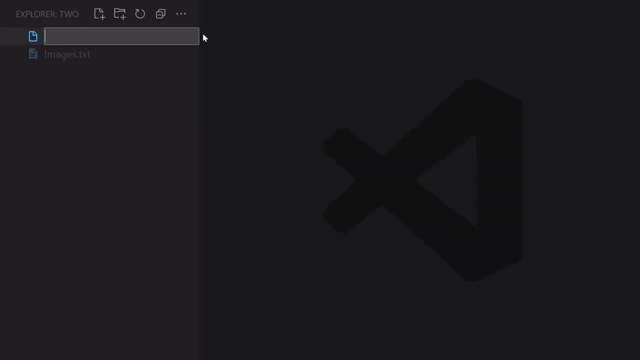 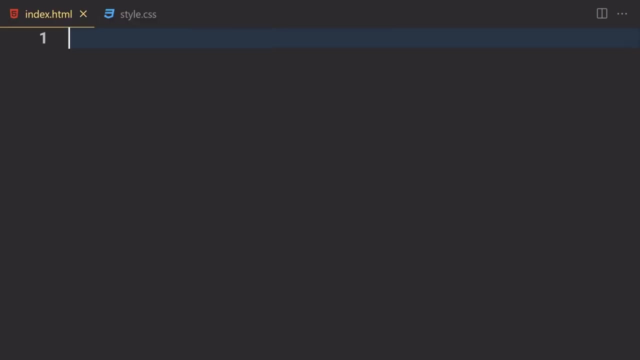 so let's just get into it. first of all, we have to create a file, give a name of like indexhtml. now let's just create another file, give a name of like stylecss, and now let's just write or doctype html in it. so what do we have to do? i'm going to just give a name of like the art, and i'm 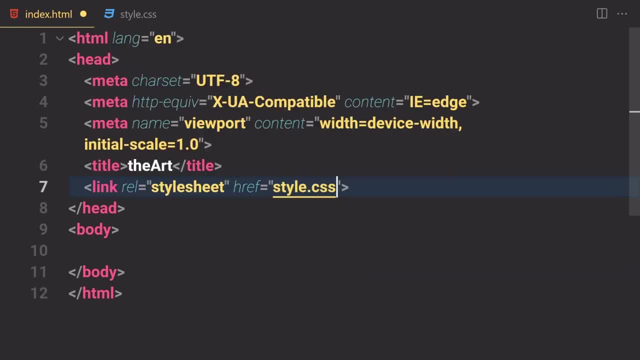 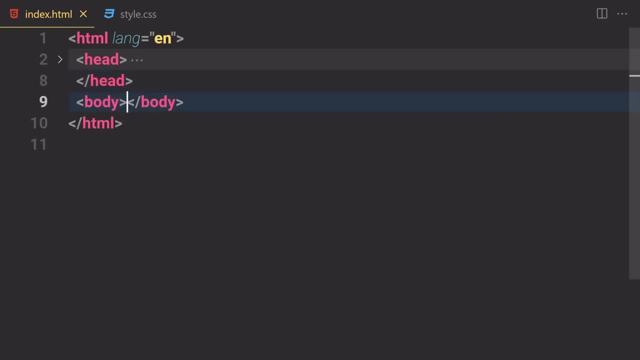 going to also link it with my css file, okay, so i'm going to hide this uh head area from there. right click on it and open it with a live server. so it will now open our file with a live server right here. okay, i'm going to zoom in a bit. so, first of all, we are going to be starting from: 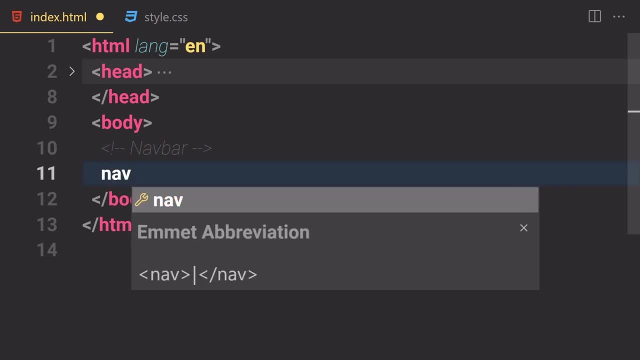 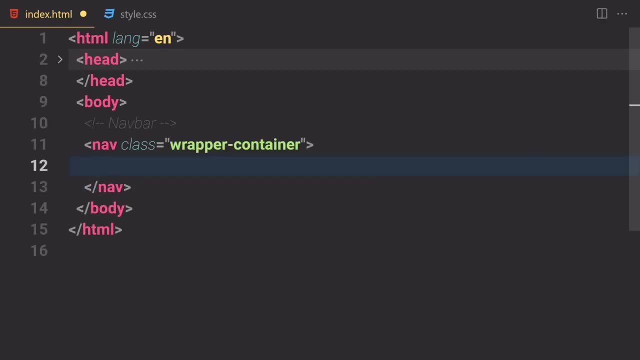 our nav bar. so what do we have to do? first of all, we just have to write our nav with a class of wrapper- uh, container. okay, so we are going to be doing that. so inside this uh wrapper- you know what- we are going to be changing that to like some sort of a section. i guess i'm going to change. 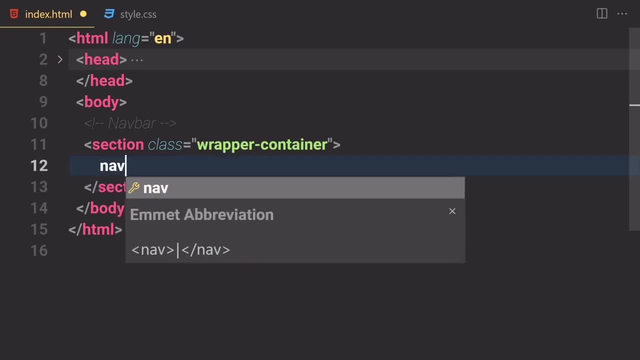 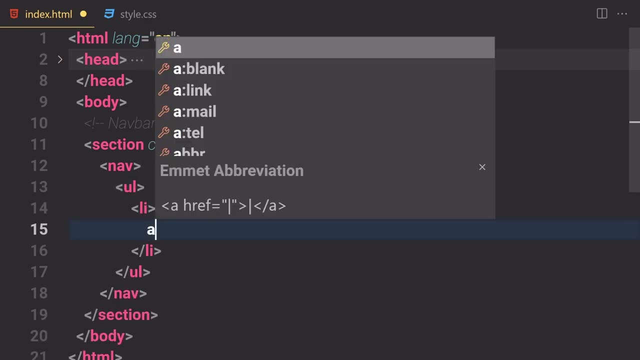 that to a section and inside this section we are going to start working on our navigation. so we are going to be writing our nav opening tag and closing tag. inside this nav we are going to be writing our ul and li and then our anchor tag, and it will go to nowhere. and here we are going. 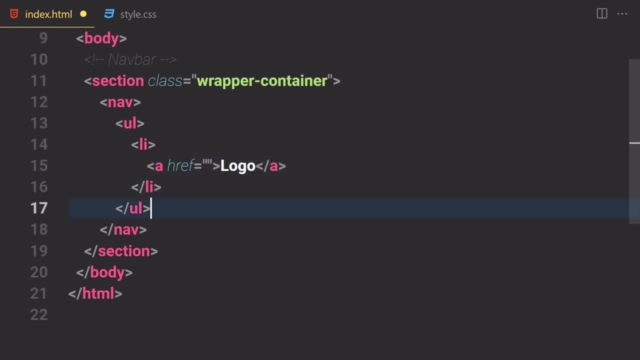 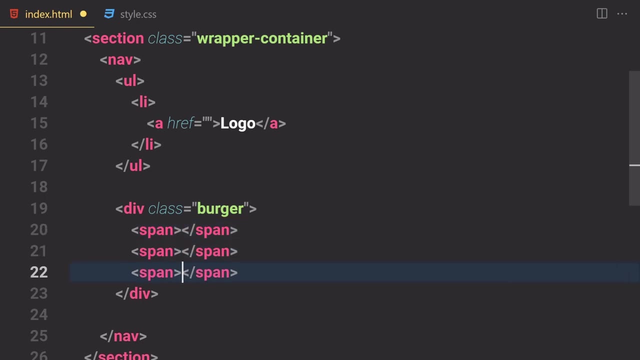 to be placing our logo right there and underneath this ul. right here, we are going to be writing our uh burger menu, right here, okay, so we are going to be writing our span and we need three of them, so, if you save our file, so this is how currently things looks like and we don't have their burger. 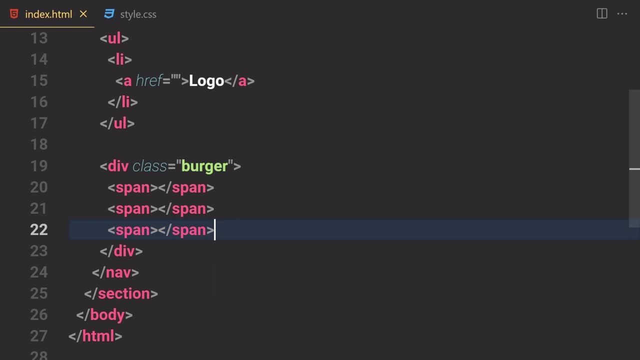 that's because we don't have any content for that anyway. so now let's jump into our style sheet. and now let's just start a bit of styling for our project. so first of all, we are going to be writing our resets for our projects. so what do we have to do? we have to select everything. 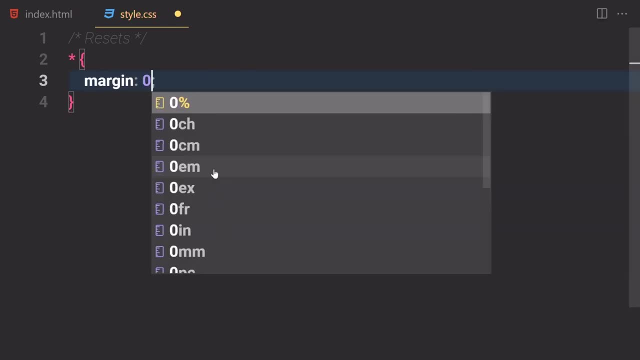 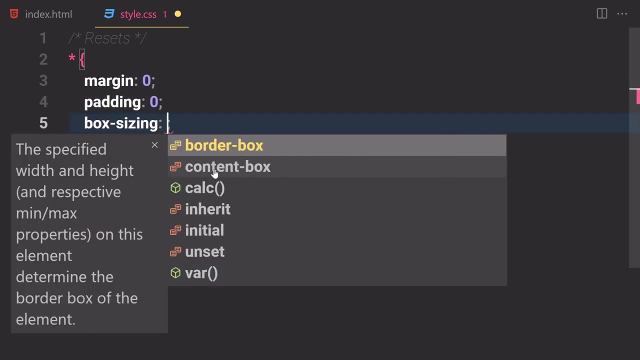 and remove the margin- not a max resolution, but now let's just select our margin and it will be zero. and padding will be also zero, not paired, but just padding will be also zero. and box sizing: i want to set that to like a border box. so if you save that, everything is working the way we expect. 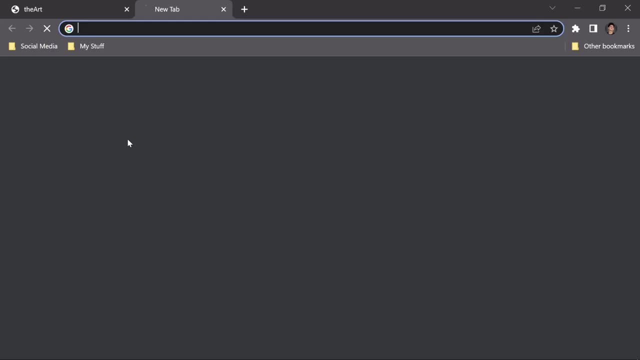 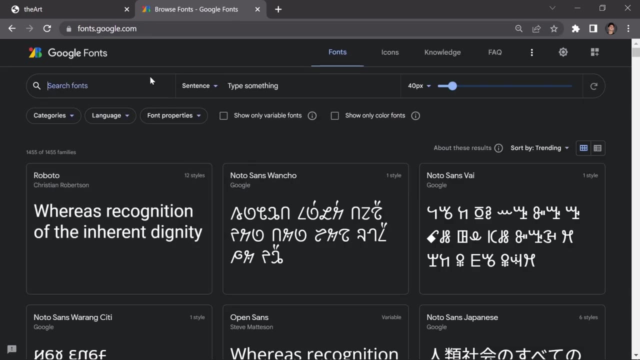 them to work all right. so what else do we have to do? we have to go to our fontsgooglecom site and here we have to grab a few forms. the first font we are going to be getting is something called open sense. so i'm going to just search for open sense. so let's just click. 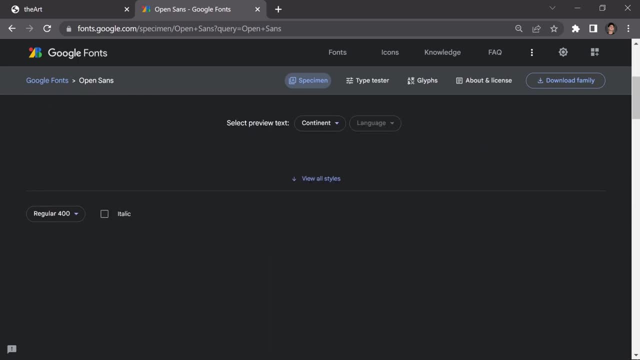 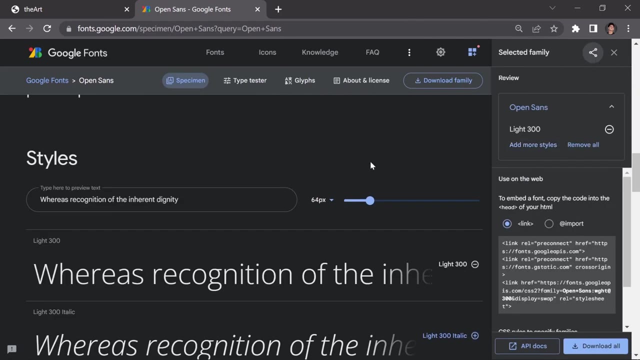 on this one and get the font width of that is like 300 pixel font width, all right, so i'm going to just select this first one. yeah, i'm going to just select this first one, not italic version, but just a regular version. so now what i'm going to do? i'm going to click on this import right here and i'm 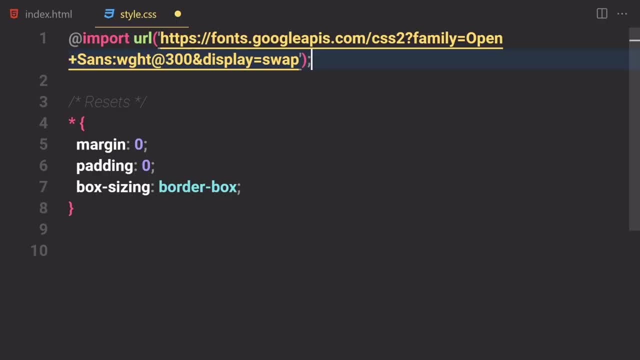 going to paste it at the top of the file right here and i'm going to also copy the font family of that. so i'm going to copy it real quick and i'm going to paste it right here and i'm going to comment it real quick. all right? so that's just kind of a basic setup. so now let's just start. 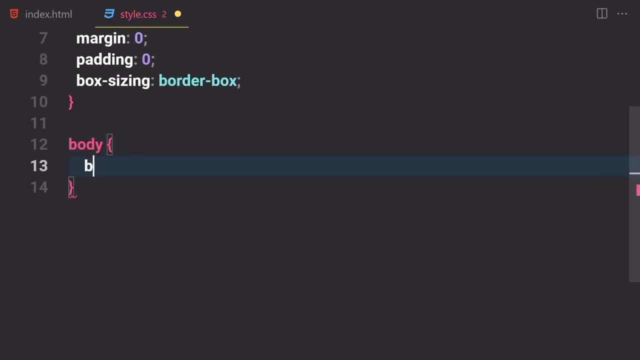 working on our body. so we are going to be first of all writing a color for our body. let's just write a, bg and c for background color and we are going to be started working on our e, b, e, a, e, 9. okay, so this is kind of the color which you are going to be using for our body. 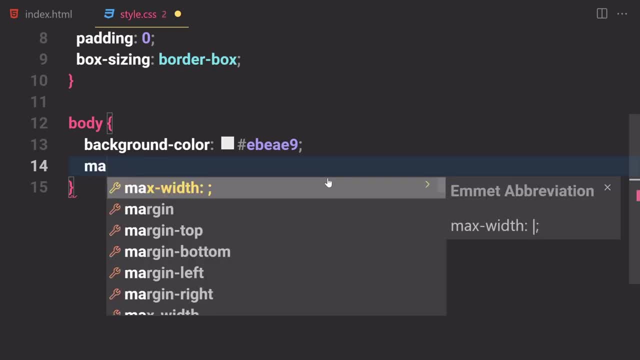 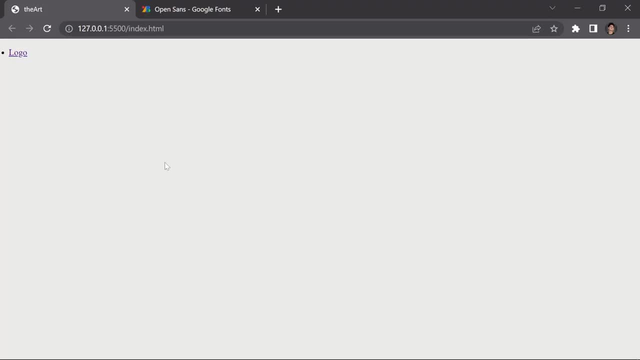 let's just write a font family of one, so this is our font family of the day, and let's just provide a margin. or yeah, i'm going to go with the margin real quick, so i'm going to just provide a margin. let me just write a margin of one rim right here. so if you say our file, so this is how. 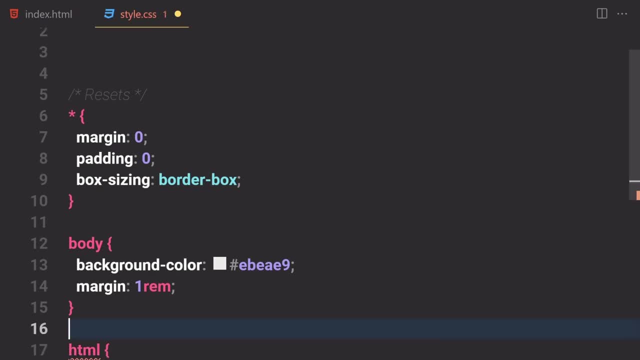 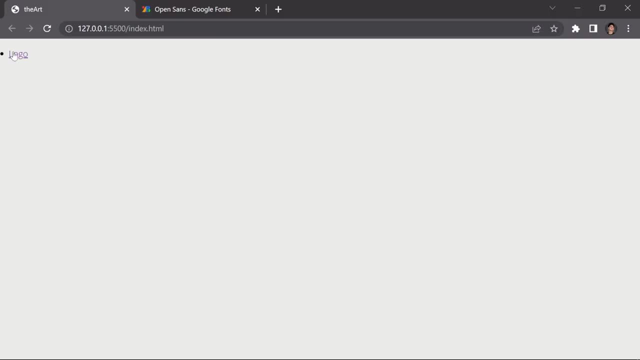 currently things looks like for now. so now let's just start working on our html. so i'm going to just select their html and i'm going to uncomment this line and i'm going to copy that. and here, what do we have to do? i'm going to just write like a font family of that. so if you say our file and 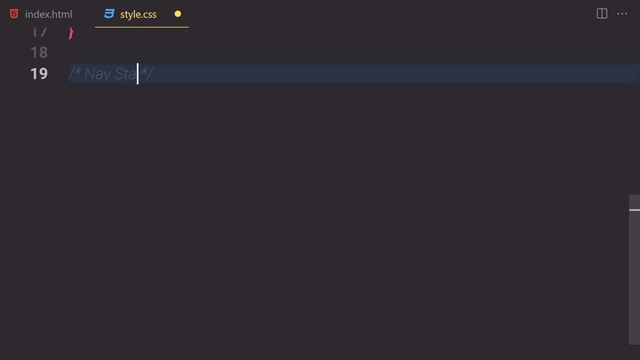 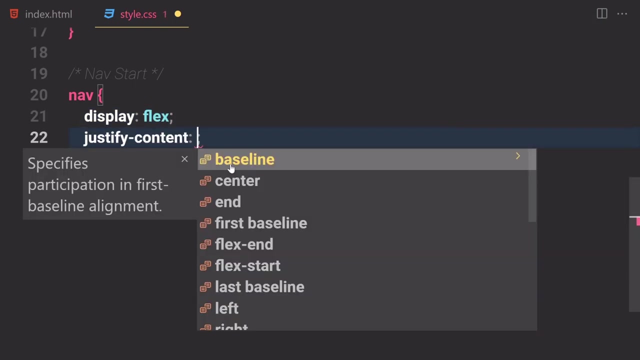 our navigation. so i'm going to just write like a nav: start, okay, start. and now inside there we are going to be selecting our navigation. first of all, let's just write a display of flex on it. justified content will be set to space around- uh, not around, but between, because you want a little bit of 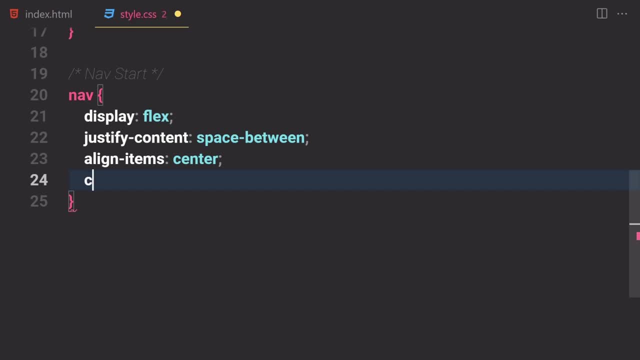 spacing. so align items will be now set to center and color will be set to totally white, and also padding i'm going to give like 20 pixel all around and margin bottom will be just five frames. so if you save there- and this is how currently it looks like right now, and here you can also see that- 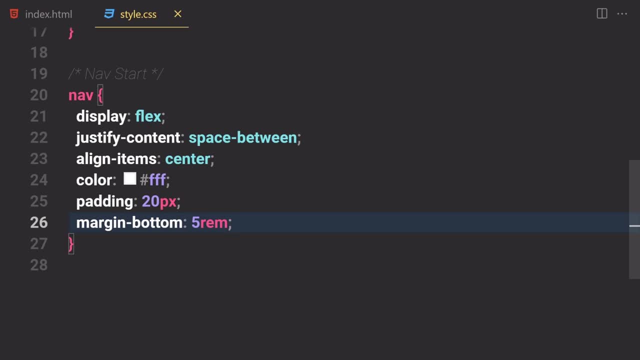 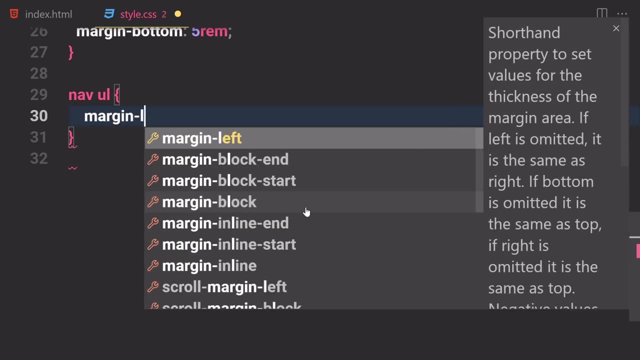 bullet point anyway. so if you want to remove them and we want to provide all the forest styling, so first of all let's just select or ul inside this navigation. so we are going to be selecting that. and now let's just write a margin left of five frame and list style will be now set to none. so 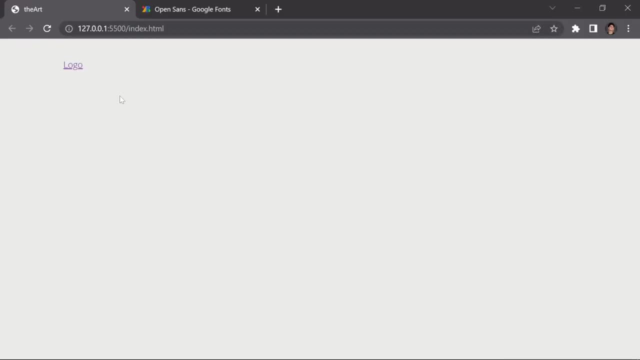 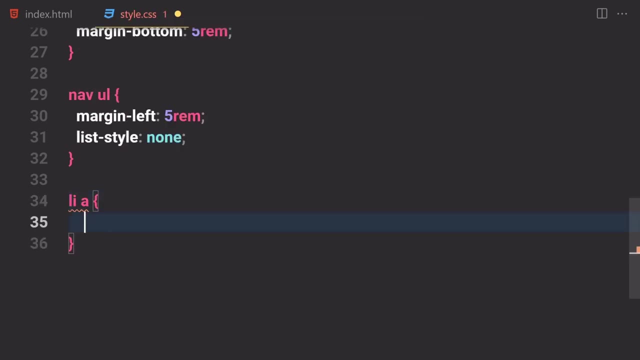 if you save that and this is how it looks like for now: now let's just remove this ugly border border from it. so now let's just remove that real quick. so i'm going to just write like: align and then anchor tag. so we are going to be writing a text decoration of none, so that you want to. 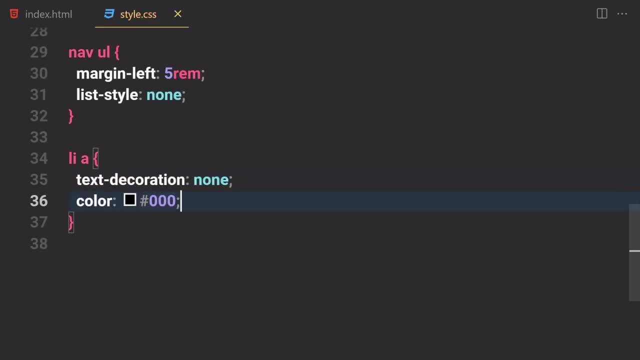 remove that decoration and color will be set to totally black and if you save that- and this is how currently it looks like anyways, so we are now totally done with that. now let's just work on our burger menu. so i'm going to just write a navigation and i'm going to select my burger. 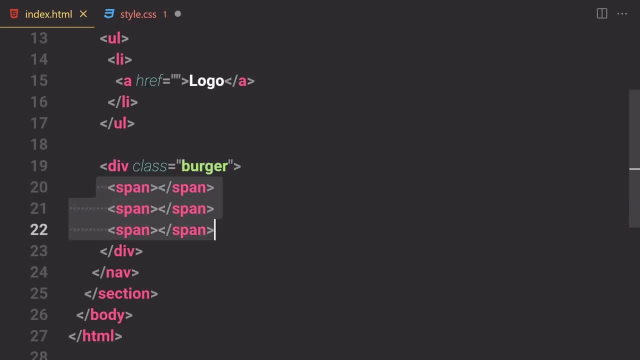 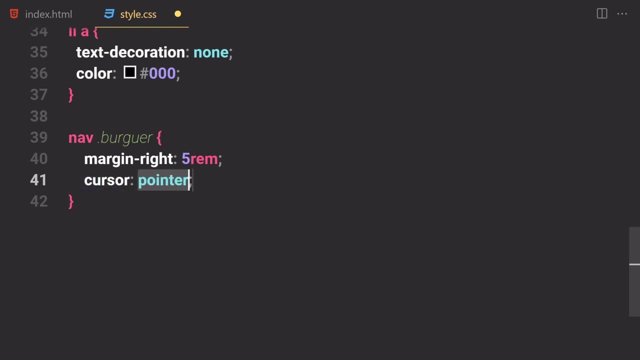 which is this class right here and here inside this burger. we have three spans right there anyways. so now we select that here we are going to be just writing a margin right of five frames and cursor will be a pointer for all of the burgers, or the spam to be precise. we are going to 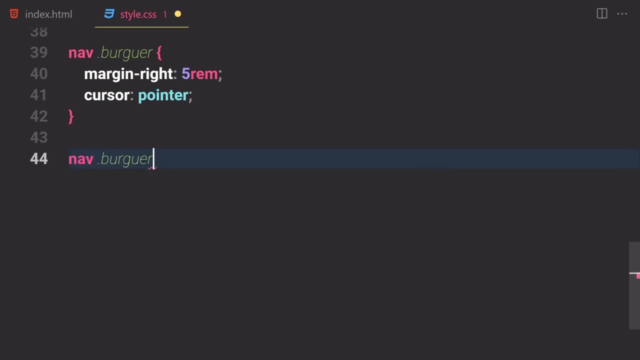 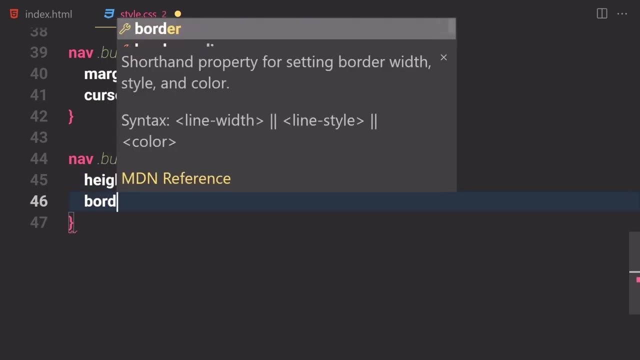 be using navigation, first of all nav. then we have word burger, and now let's just select our span, and here we are going to be giving a little bit of height, like 400, not 400, but just a 4 pixel. and now let's just write a border of two pixels, solid and totally black. 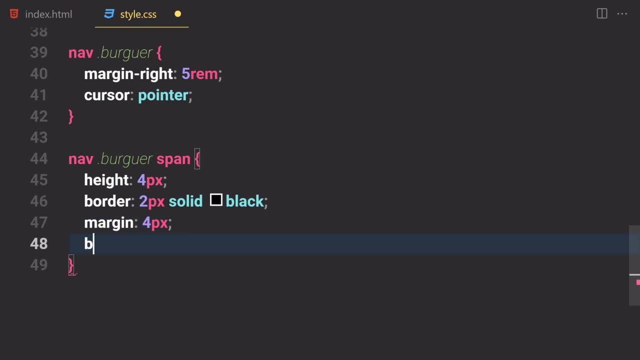 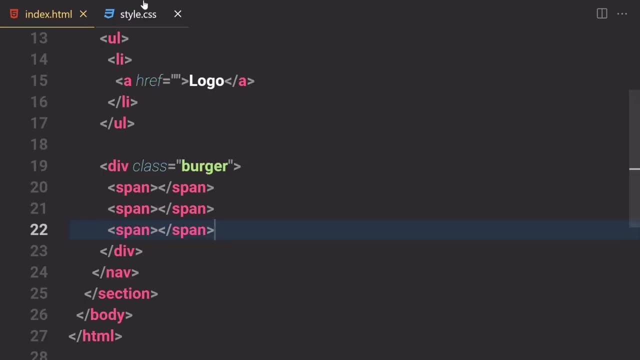 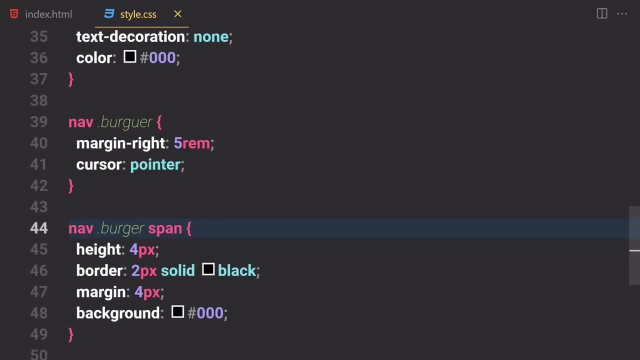 and now let's just give a little bit of margin all around, like four pixel, and background will be totally black. so now, if you save that- and i guess you cannot see that- i don't know what's going on. all right, so we have our navigation, then we have b-u-r-g-e-r and now, if you save that, yep, we are. 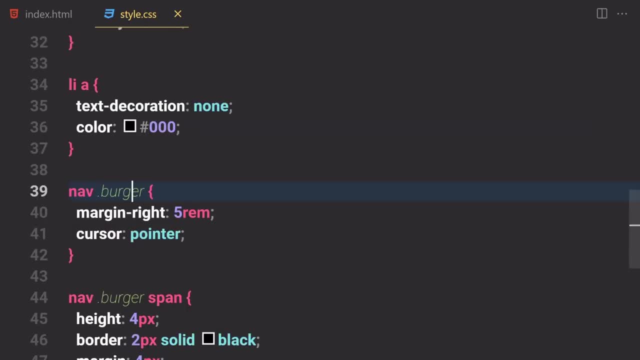 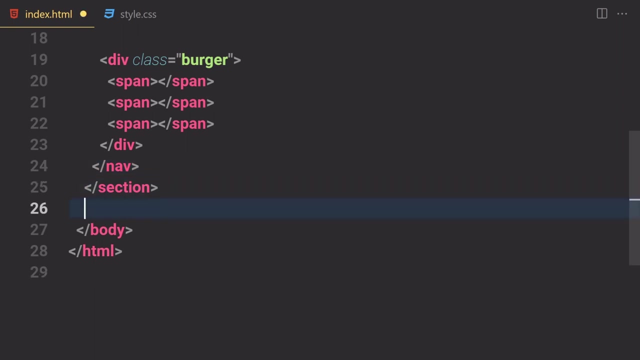 getting it. and this is also a burger. yep, both of them are now currently working. now, the next thing which we are going to be doing is that we have to start working on our header area. so here i'm going to just write, like a navigation, n and yep. save that. and here i'm going to also write a navigation. 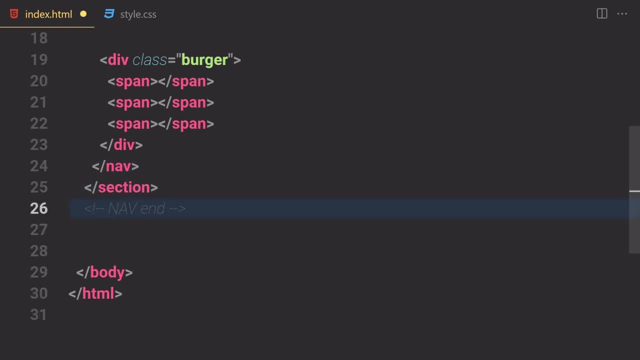 n nav end. yep, that's cool. so for header. now let's just start working on our header area. so i'm going to just write like a header area in here, or here area, whatever you want to call it. so here i'm going to just put like header opening and closing tag, and now let me just write h1 with a class of 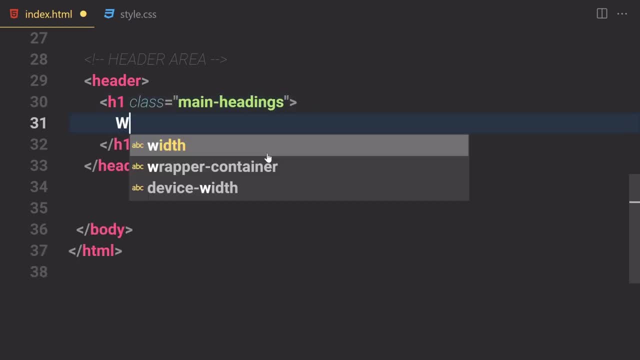 main headings: okay, so inside this h1, we are going to be writing first of all what, and then br, and then, underneath this br, we are going to be writing: is car, and then art. okay, question mark. underneath this h1, we are going to be writing our paragraph with a class of 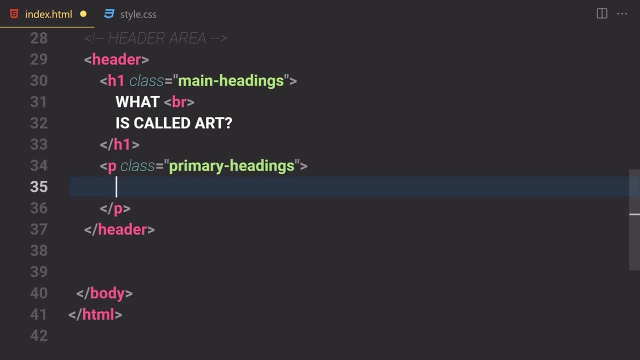 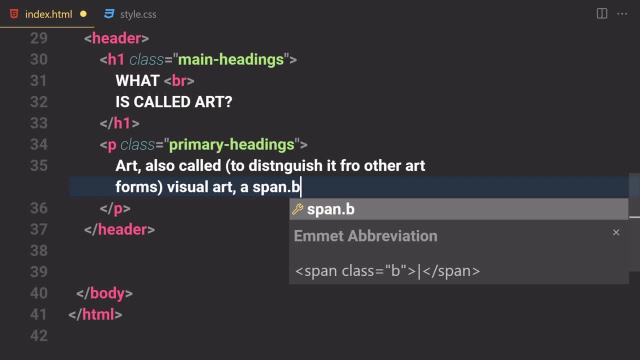 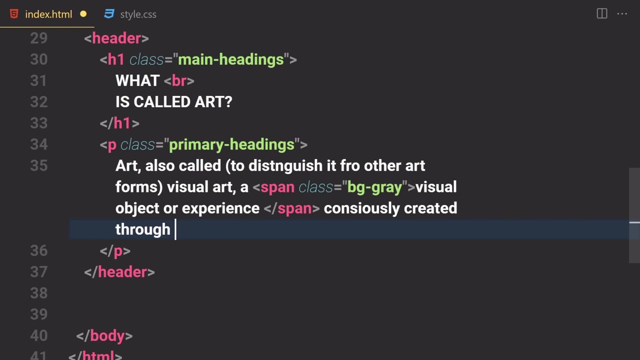 comma, comma, span. and now i'm going to give him a class of bg, of gray, okay. so visual object or experience and yep or span will end in here and now. let's just write concisely: created true and not part, but through an expression of skill or imagination. okay. so now, if you sell that, this is how it looks. 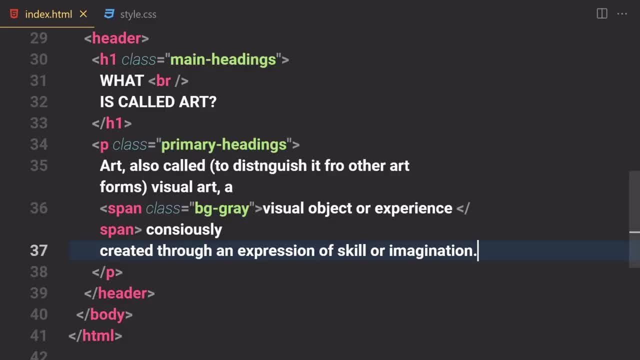 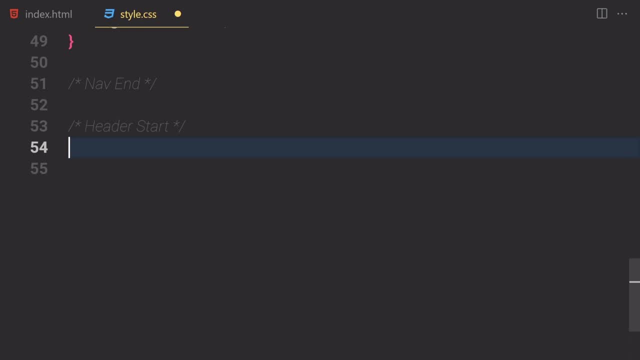 like i know it's awful. now what else do we have to do? now let's just go towards styling, and now let's just tie a little bit. so here what i'm going to do: i'm going to just write like a header start, and now let's just write our header and i'm going to give him a little bit of. first of all, let's. 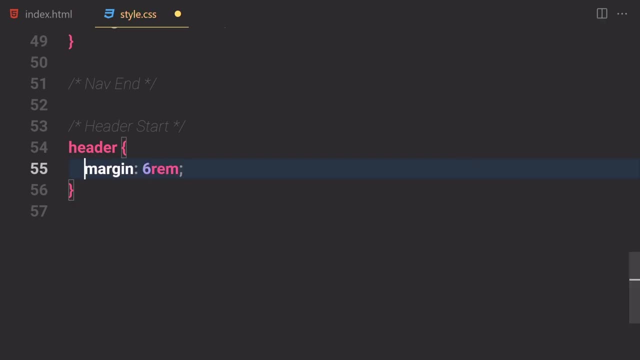 just select record correctly. i'm going to give a margin of six rim from all around and now let's just select our main headings. okay, so now we selected that width will be just a 50 percent font size. i'm going to just increase that to like three rim and, yeah, i'm going to also select my primary headings right now and 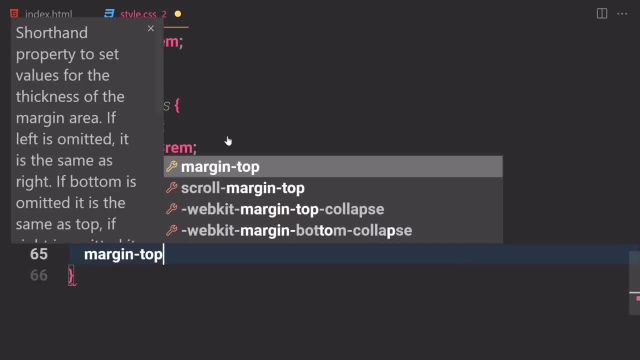 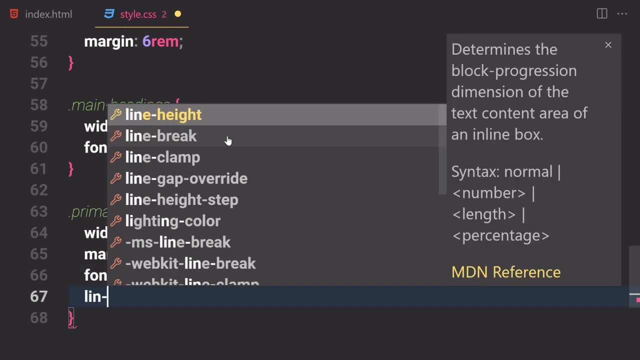 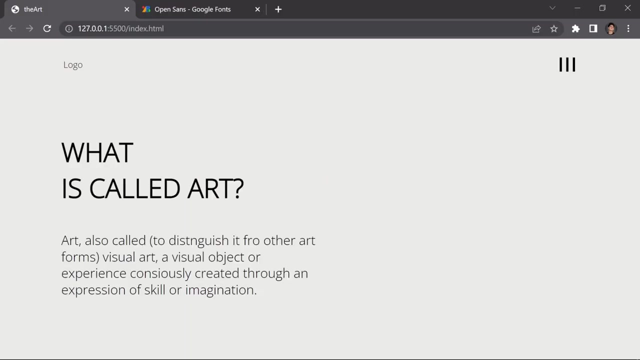 i'm going to give my width of like 50 percent in here. margin top i'm going to give it like three rim and font size will be just like 1.5 rim and line height i'm going to give him like 30 uh pixel. just a 30 pixel will be fine. so if you save that- and this is how currently things looks- 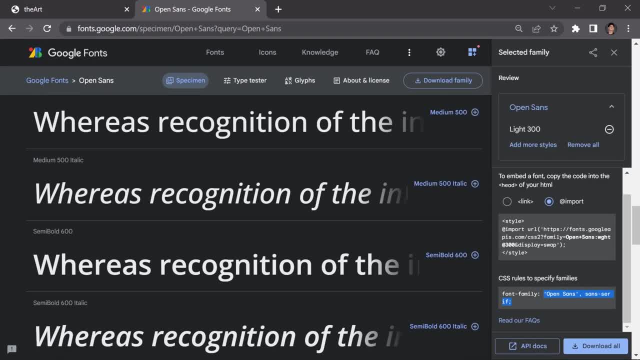 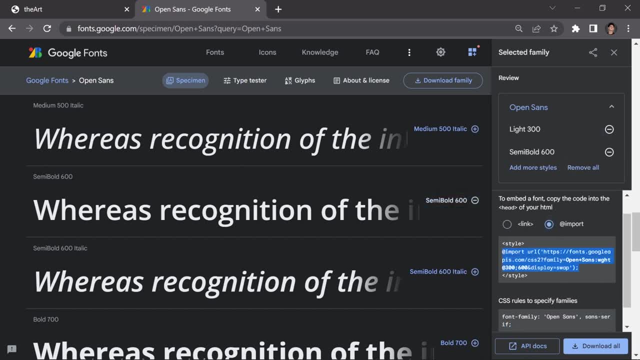 like. so if i want to make that board, you know what? i'm going to also get some sort of a board version of it. so i'm going to also click on that and yep, now i'm going to copy this one copy there and go to the top, replace it with the other one. 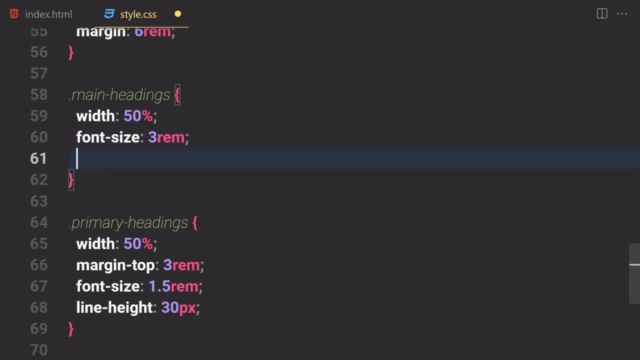 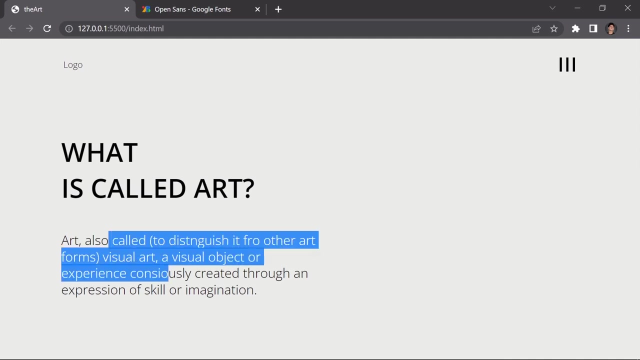 now go to the bottom and change this one font rate to be like: uh, which one was there? yeah, just select like 600. so i'm going to just write 600. so save our file and this is how it looks like. so first of all, save it. yep, this one is a little bit darker than this one and this one is looking cool all. 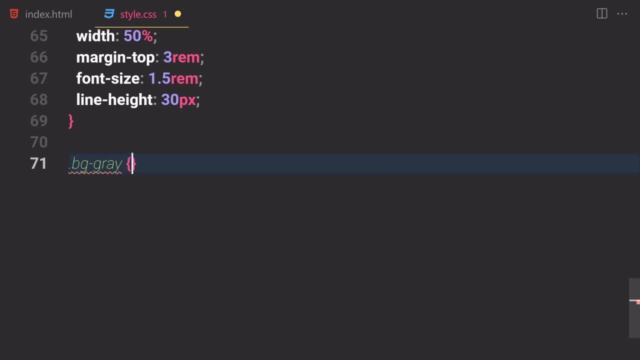 right. so now let's just write there: bg of gray, uh, which is this pen right here. so it will just change the background color to be like some sort of a grayish color. so i'm going to just give a background color of rj gb. let me just write it: rgb of 53, uh, not 50, but just 53 and 53 and 53. okay, so this is the. 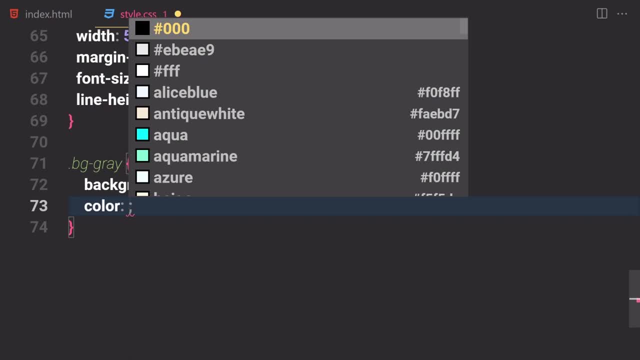 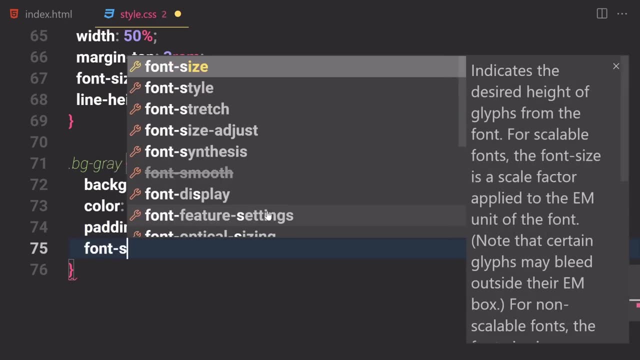 background color which you are going to be using, and color will be now set to like totally white and padding. i'm going to give him like two pixel for top and bottom and 10 pixel for left and right, and i'm going to also change the font rate to be totally bold. so if you save that- and this is how- 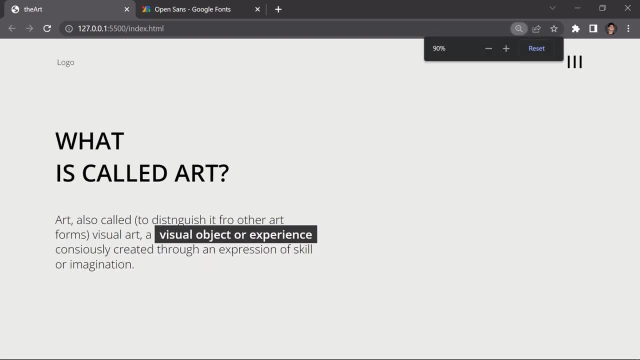 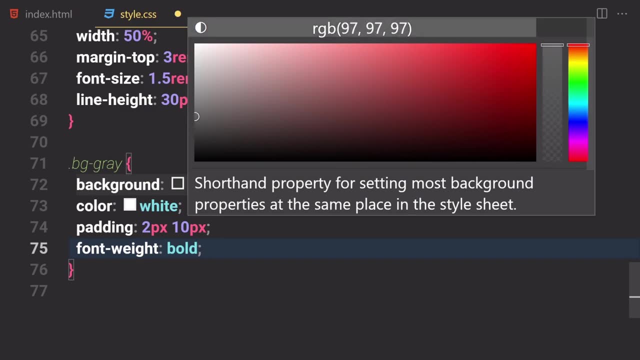 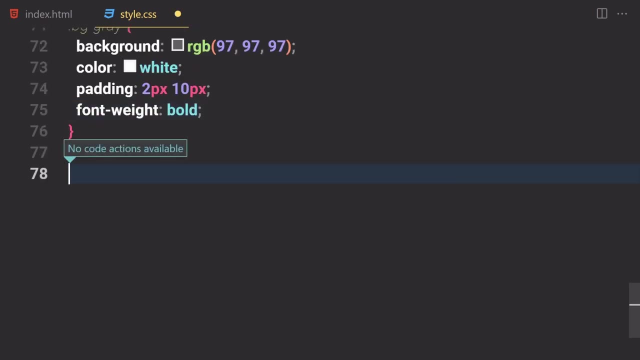 it looks like right now and you can play around with that if you want to like. so i guess that would be fine. yeah, oh, you know what i'm going to make it a bit subtle, like so: yeah, that's fine, you can play around with that if you want to. but that's kind of a call to action. so here i'm going to just write. 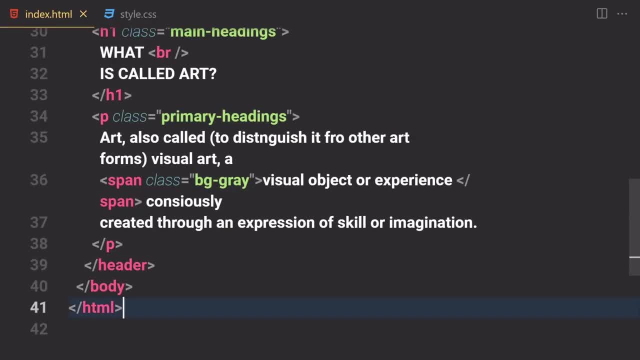 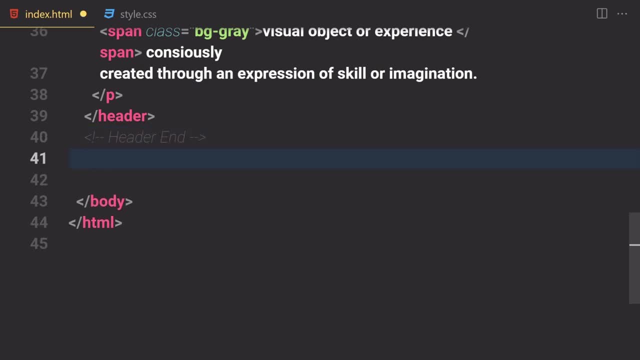 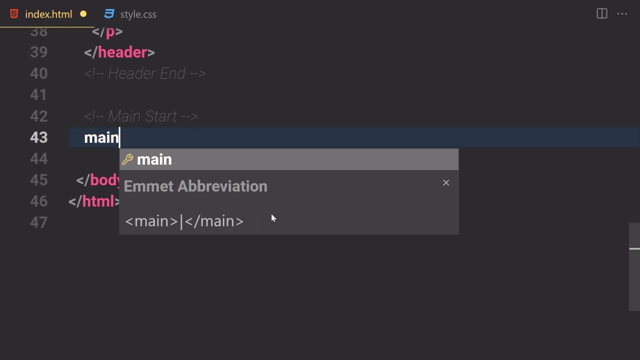 like header n, and here i'm going to also put a header and comment in here. so let's just write a header n and now let's start working on our main area. so i'm going to write a main start and now let's just select our main area and inside this main area we are going to be just placing our images. so i'm going 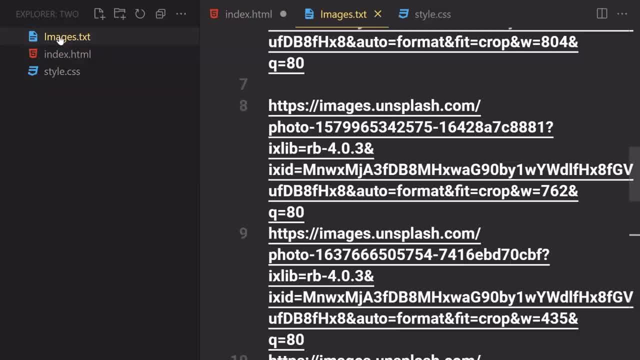 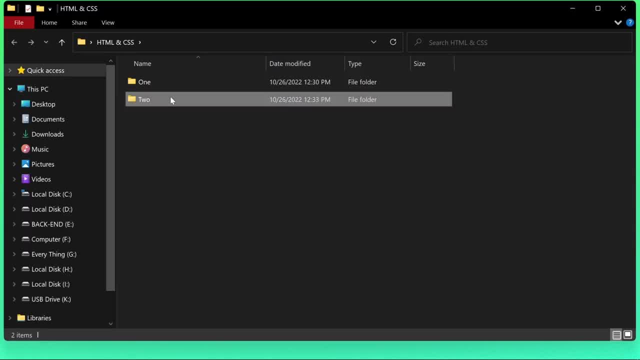 to just write image and now let's just select all of our images from here. uh, okay, so it's looking a bit clearer. i'm going to go ahead manually, like: i'm going to just open my html and css, click on that and i'm going to select our images from here. all right, so i'm going to select my. 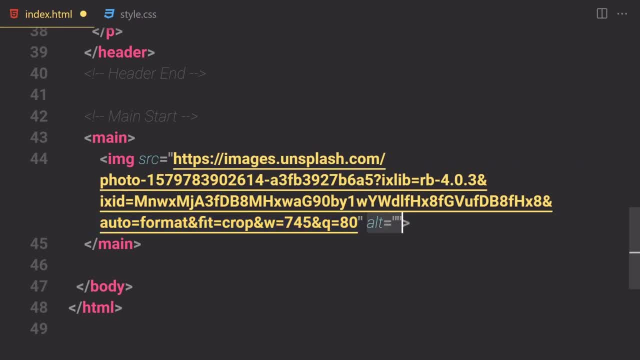 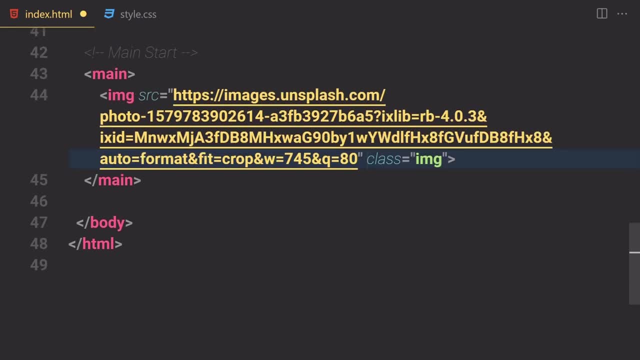 first image. i'm going to place it right here and we're going to be removing this art attribute from there and i'm going to also give him the class of img. oh you know what first? yeah, i, i get that would be fine. i guess that would be fine. so let me just write img one more time with the class. 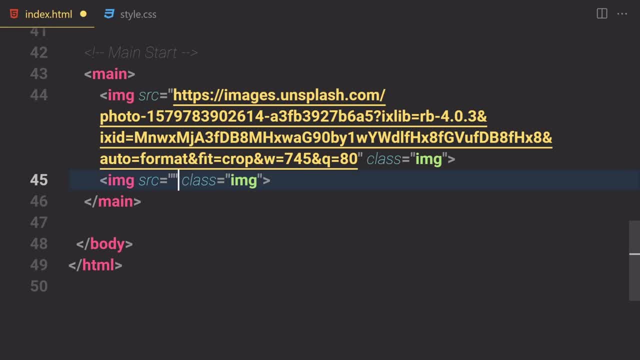 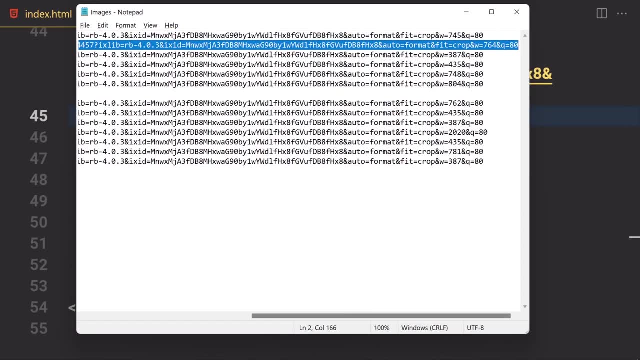 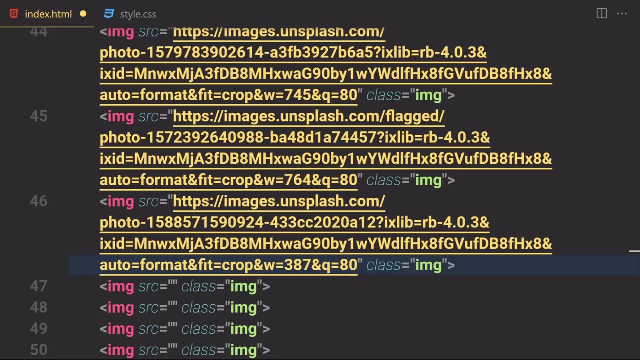 of mg. okay, so i'm going to remove this alternative text from there and i'm going to duplicate that a few times like so, and now i'm going to just replace it with these images. so i'm going to copy that, paste it and copy that and paste it right here. let's just copy that other one, i guess. 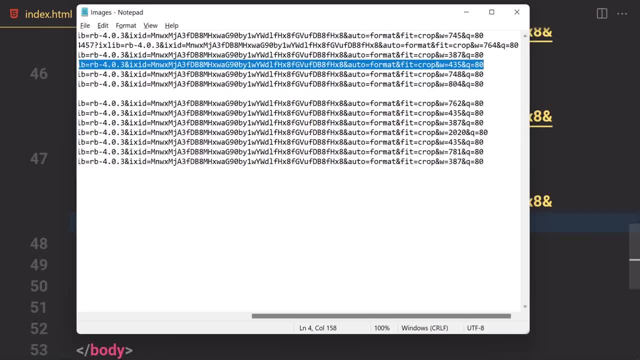 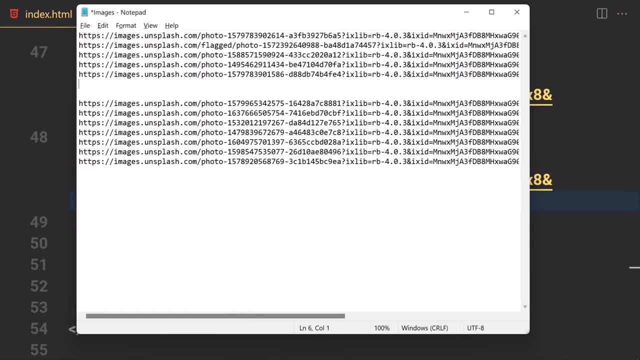 this is on the fourth one and let's just paste it in here. and, by the way, if you're wondering, like, where am i getting these images from? so i get all of these images from unsplashcom. i don't own these images, so if you want to get all of these images which i'm using for this project, so you 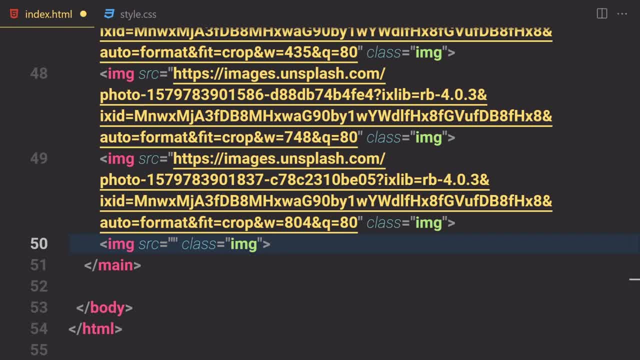 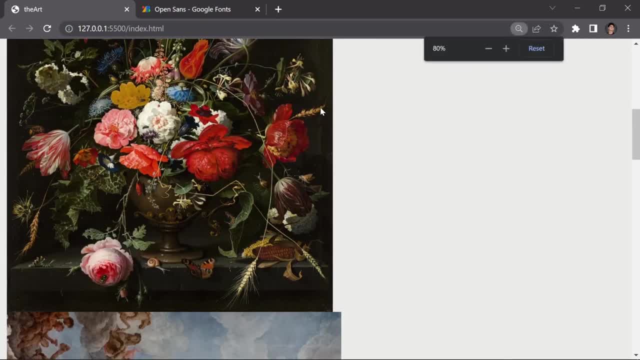 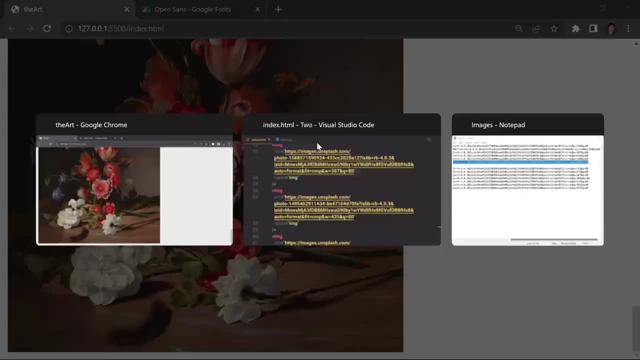 should either go to my dm repository and download it manually, or you can just go to the description area. you and you will also find their images out in there. and now here are my images. so these are the images which i'm going to be using for this project. so now let's just style that a bit so. 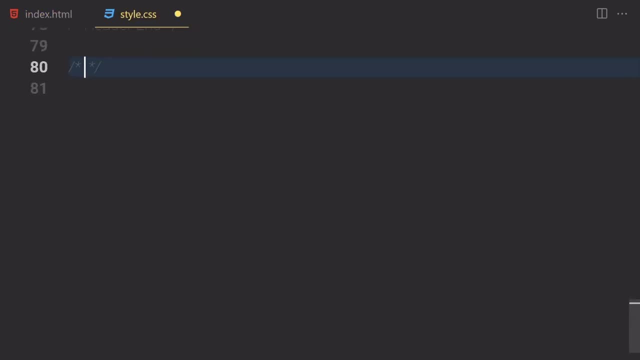 i'm going to go to my stylesheet real quick and here i am going to write my main start. okay, so i'm going to select my main and now let's just write a margin: 0 for top and bottom and forum for left and right display will. 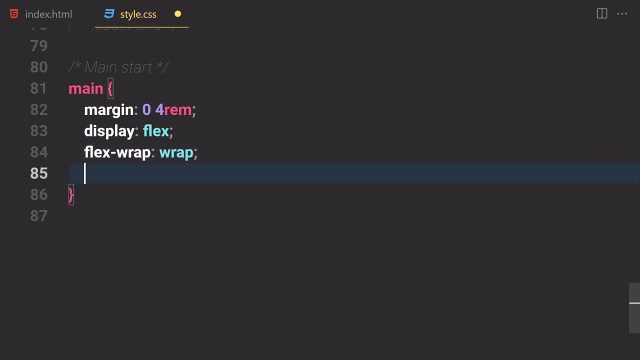 be totally flex and flex ramp will be now set to wrap justify content. uh, justify content will be now set to center and margin. i'm going to give a little bit of margin of 40 ram, not remember pixels. so if you save that- and this is how currently things looks- like clutter, uh. 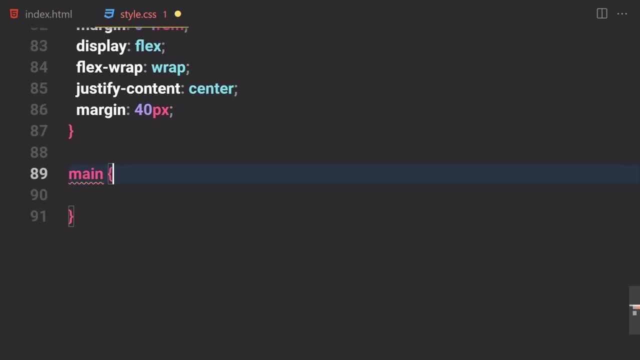 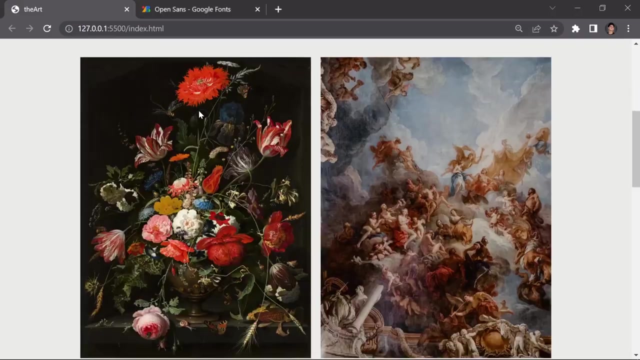 so now let's just select that image. so i'm going to write main and now let's just select that image. so img and all of these images have this class of img right here. so now let's just select that and give them a width of like 40 percent, and i'm going to also provide a margin of 10 pixels. so if you 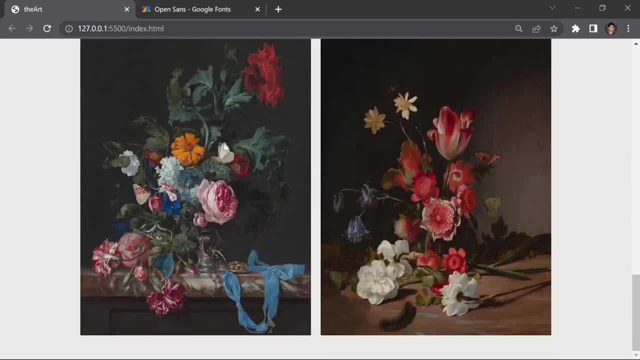 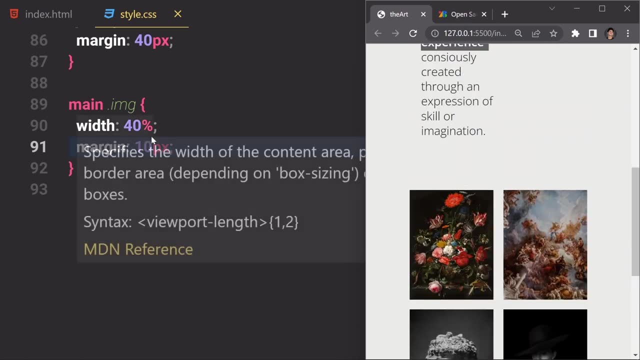 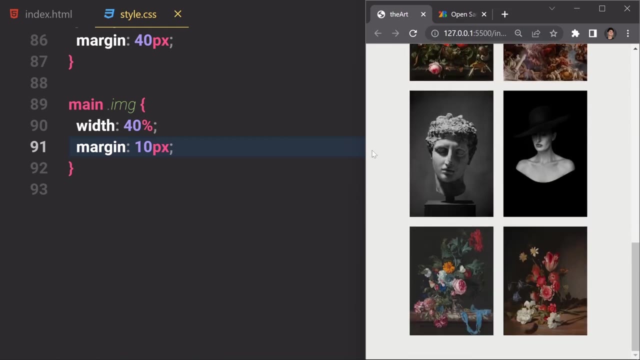 save that and, yeah, that's looking better right now. okay, so if you just make our screen size a bit smaller, it will still look good on a smaller screen size, because we provide a width of 40 pixel- not 40 pixel, but 40 percent- and we will take care about these once we jump into the media query section. so 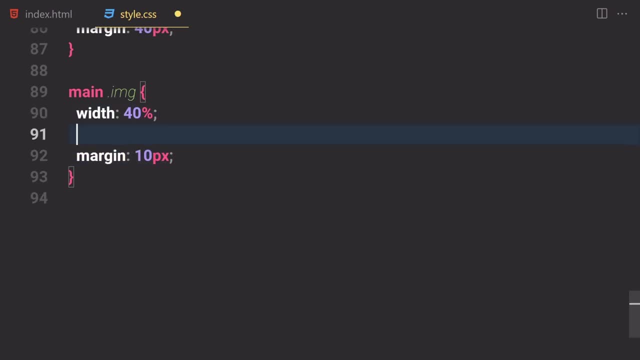 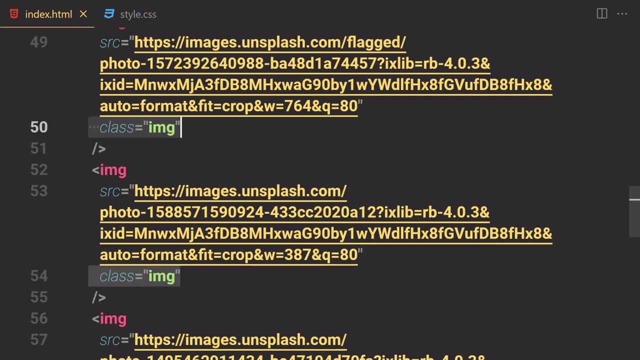 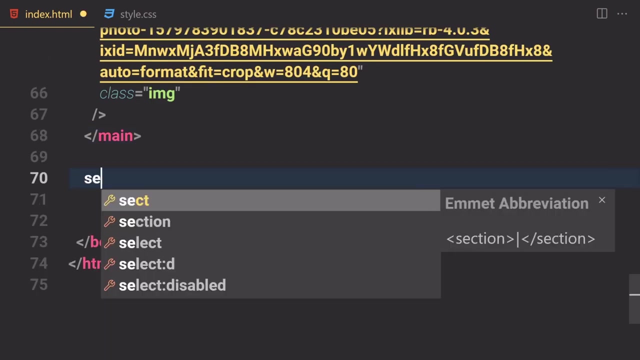 i'm going to make that a bit bigger. and now we are totally done with our um main area, so we are going to be just writing our main, uh, main end. so, and now let's just start working on our section three. but section three will be a little bit long, okay, so i'm going to just write a section with the class. 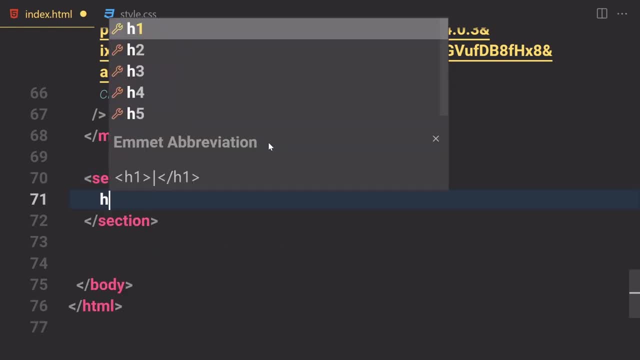 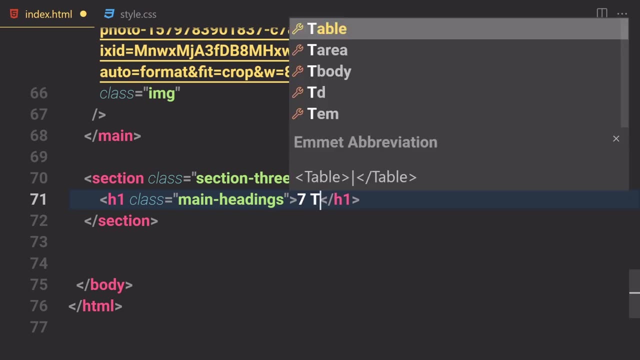 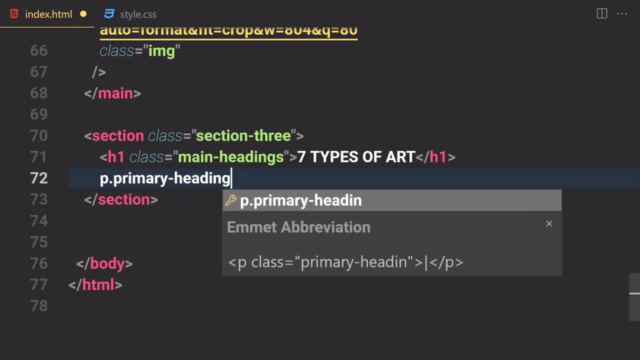 of section three. okay, so inside this section three, we are going to be writing h1 with the class of main headings, so we are now reusing that class again. so seven uh types of art, okay. so now let's just write a paragraph with the class of uh primary headings, okay, and here we have to write: 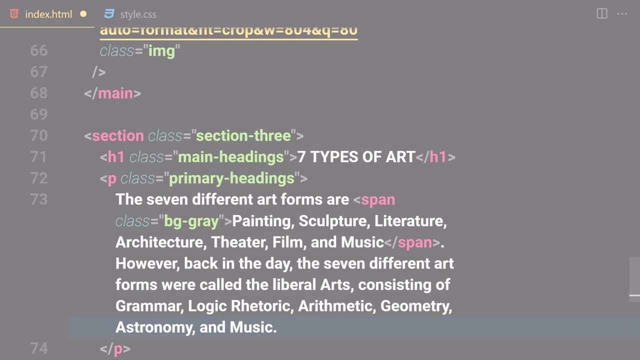 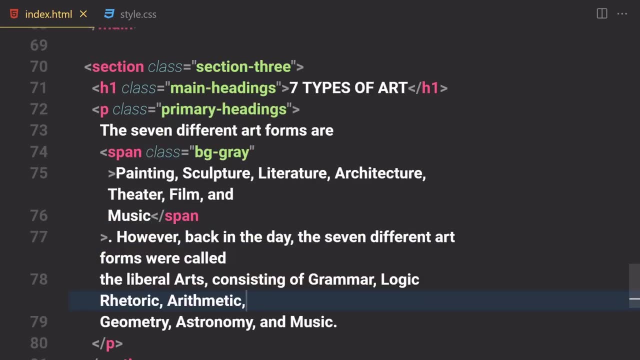 all of their uh, gibberish. so you know i'm going to just fast forward. all right, so now, if you say, all fine, so here the text i write. and now i want you to notice this: so we are using that background, gray class on this padding and these uh kind of 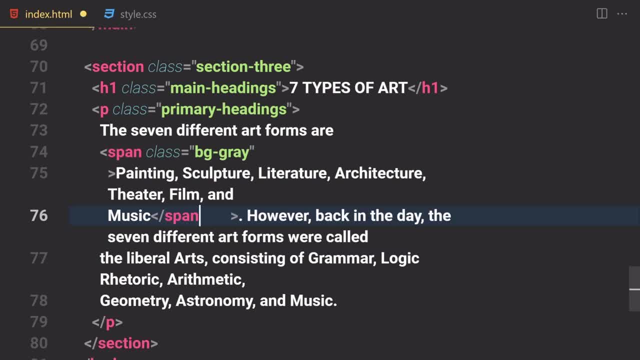 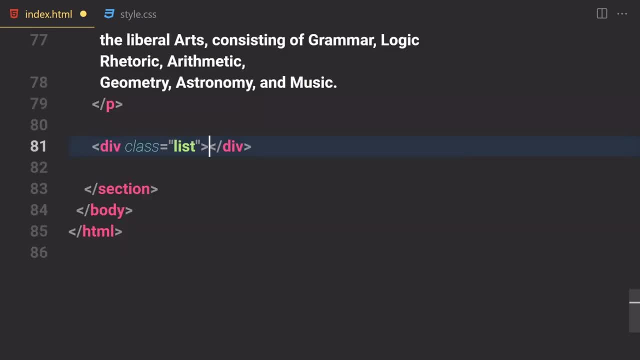 pattern area right here. so i want you to just notice that real quick. and this is all of the texts which you need for this project. so now, here we are going to be rendering our list, so i'm going to just write a list right here. inside this list, we are going to be rendering different kind of 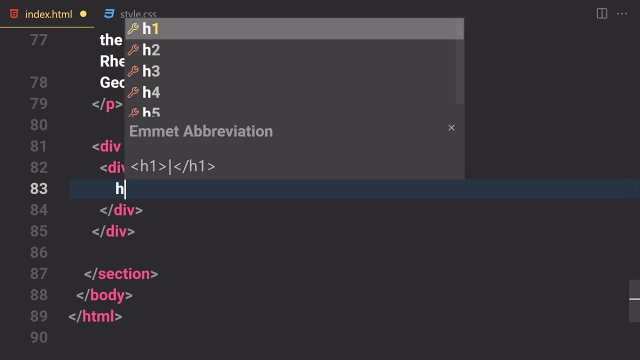 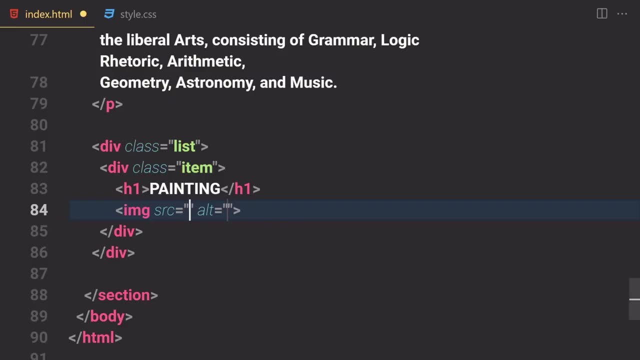 items. so i'm going to just write item inside this item, i'm going to just write h1 of painting, so painting. and now let's just write our image and i'm going to grab this image, which i have already right here. i'm going to copy that and paste right here. 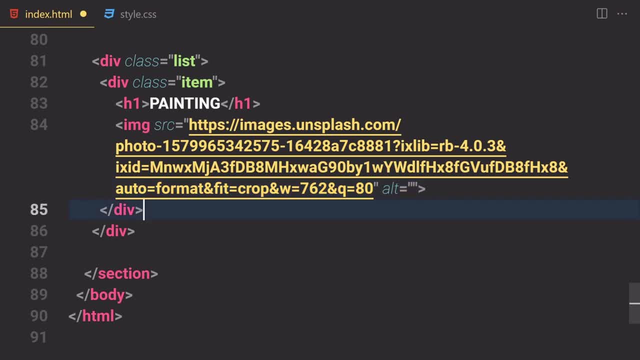 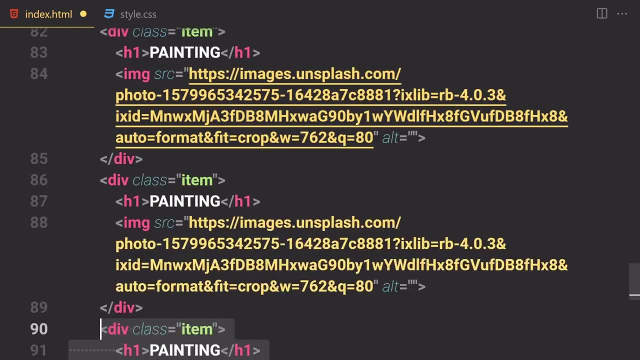 and we are. we are not going to be providing any alt and stuff, so i'm going to just duplicate this item real quick. so this one we have is our item one. then we have our item two, three, four, five. okay, so now let's just change that real quick. i'm gonna change this painting to this sculpture. 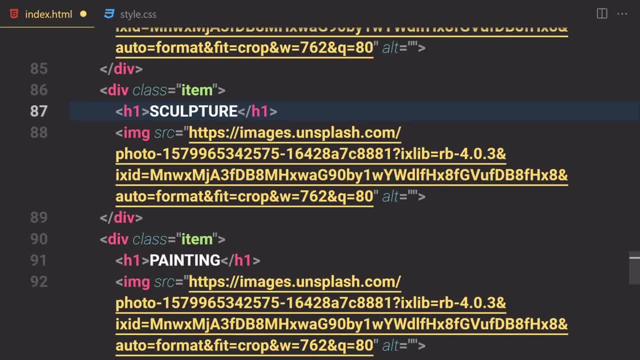 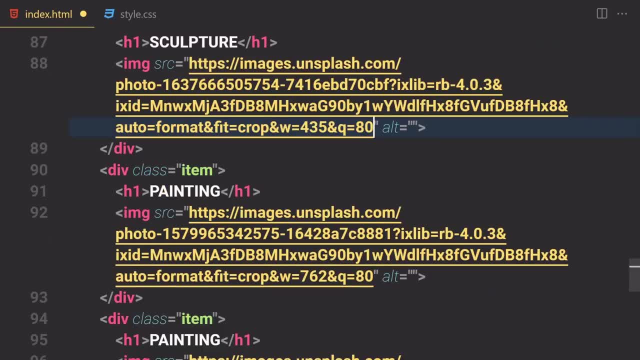 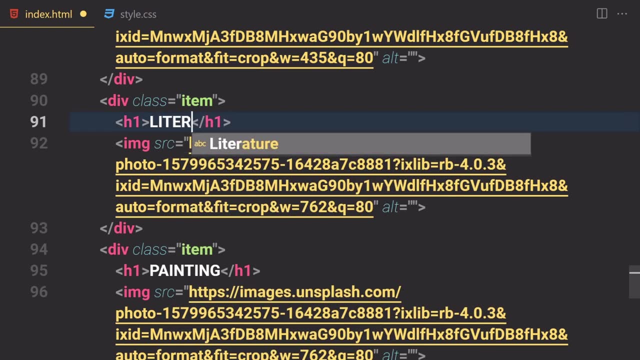 and let's just: um, sorry, i can't pronounce that name, but uh, i'm gonna change it anyways, copy it and let's just pass this link. and yeah, i also have to change that one, so i'm going to change this heading from painting to literature, so literature, and let's just copy. 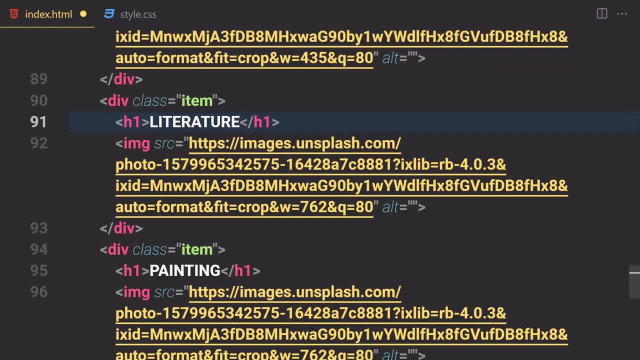 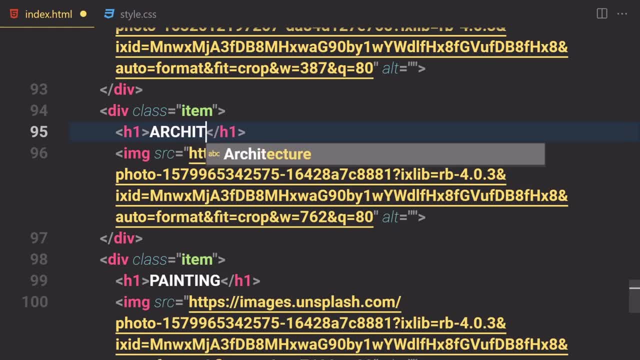 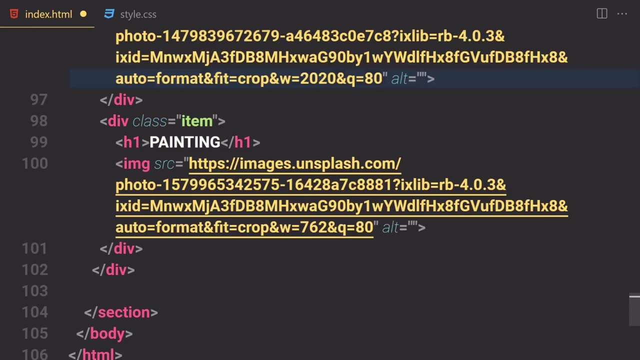 the third image right here. copy it, and i'm going to paste it right here and now. let's just change this painting to architecture, so our architecture. and i'm going to copy this image and i'm going to paste it right here. let's just change this painting and now let's just write a cinema. 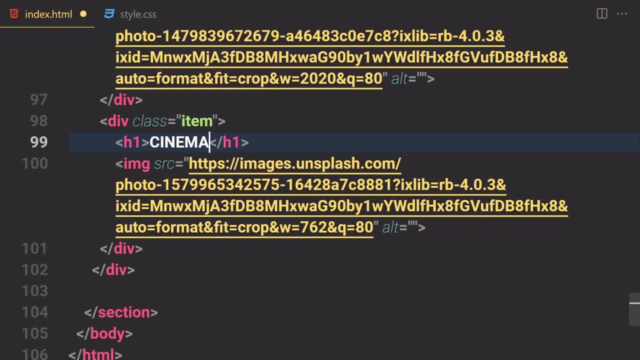 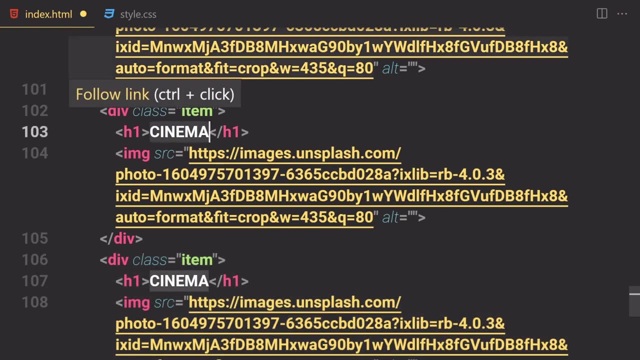 cinema in here. let's just copy this image, and i'm going to paste it right here and let me just make sure that i didn't mess up something. so okay, so we have two other left, so i'm gonna copy that two times, one and two. so change this cinema and copy this text. not text, but copy this image url, and i'm 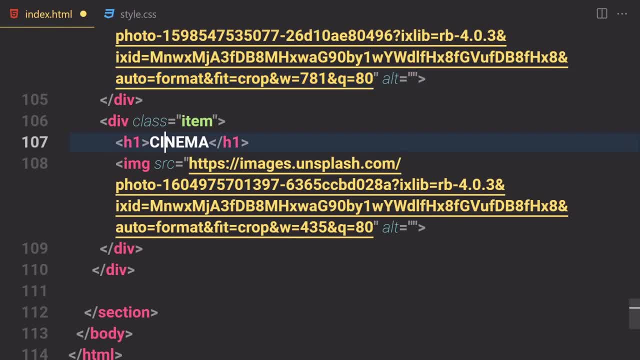 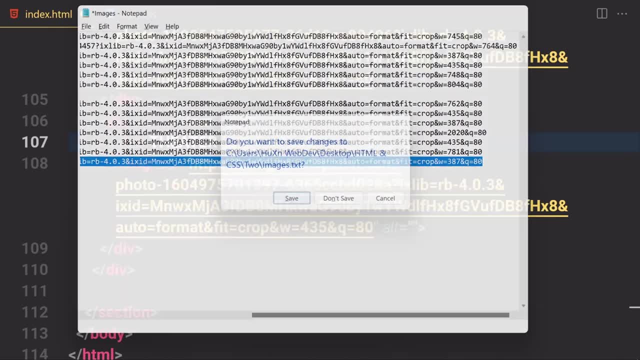 going to paste it right here. and then, finally, let's just change this cinema to theater and let's just copy this final image and we are told it done so, say bye, bye to this one, save it, and i'm going to paste this image link right there. so now, if you save that and here you can see, we have all. 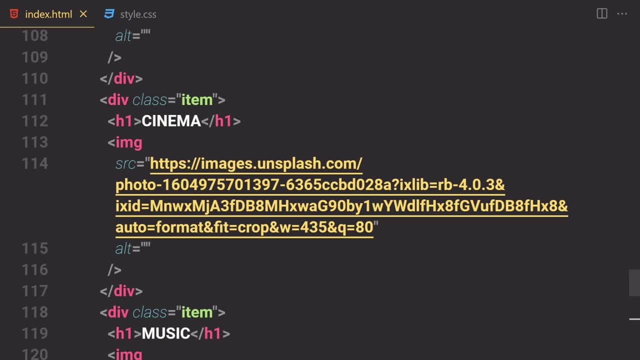 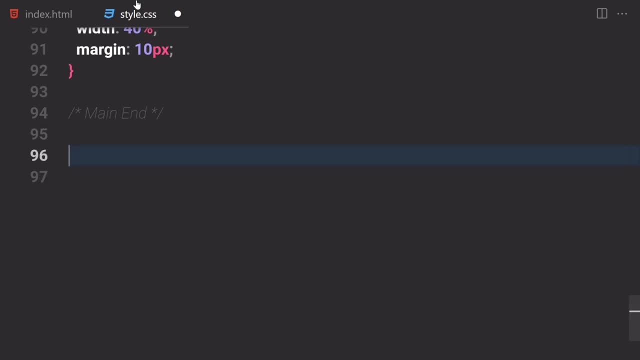 of these images and we have all of these titles right here. so now let's just get into our style sheet and now let's just style that a bit, all right. so i'm gonna write a comment for myself and i'm going to just write like: section three start, all right, and now let's just select our section 3. 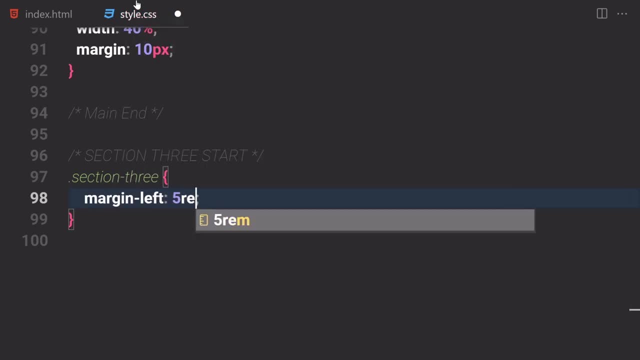 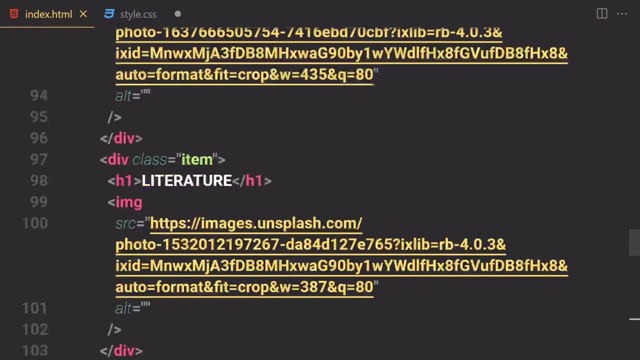 and now here i'm going to just give a margin left to be like five frame, and also let's get it or section three and primary headings. okay, so let me just write a margin of bottom of 10 rems in here and now let's just select our list, which is that huge list, which? 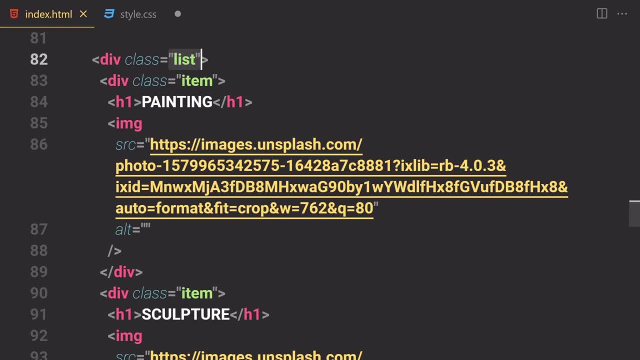 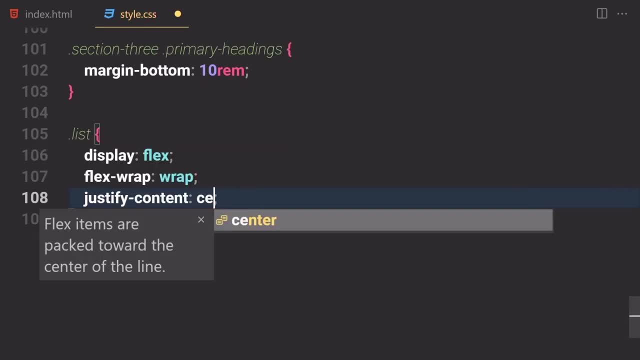 you have right here. let me just see. yeah, there we go. select that list. write a display of flex legs. wrap will be now set to wrap, because we want all of our images to wrap. justify. condo will be center. align items will be also centered. so if you save our file, 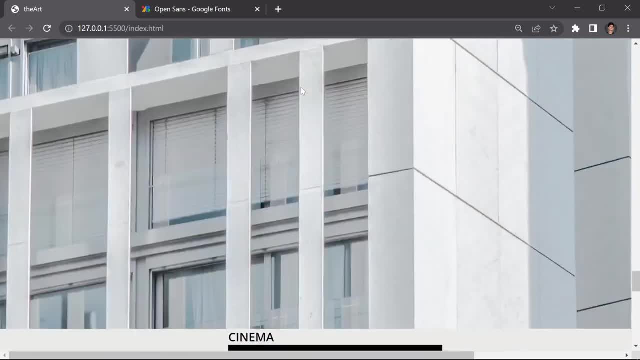 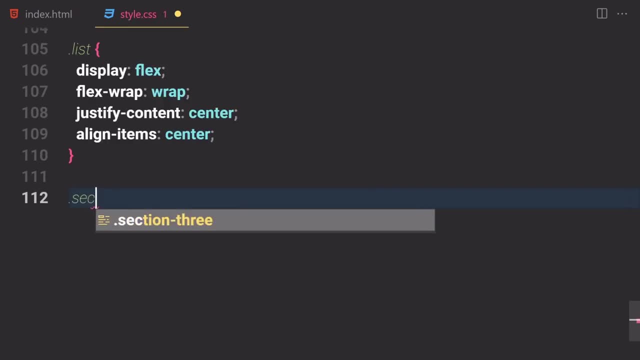 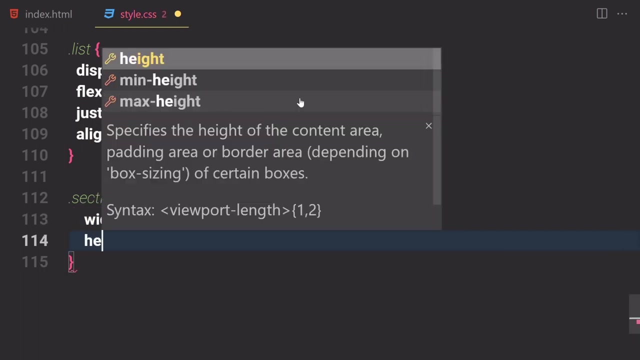 and we can see some of the images, but a lot of images are really huge and we cannot see that once. so now let's just change its heights and stuff. uh, let me just get my section three and all of the images which we have inside that section three. so i'm going to just give my width of like 400 pixel. 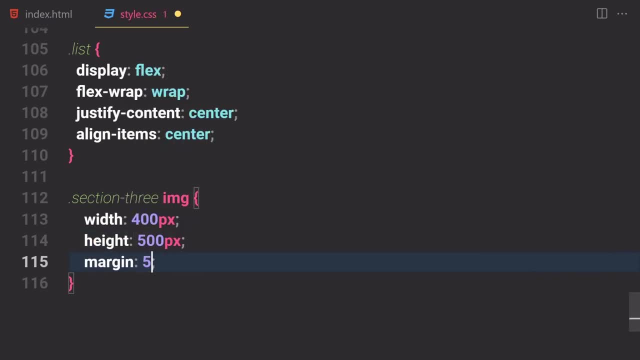 and higher, it will be just 500 pixel and i'm going to also give a margin of 50 pixels. so if you save them and, yep, that's looking better. so now let's just give a margin of 50 pixels. so if you save that and yep, that's looking better. 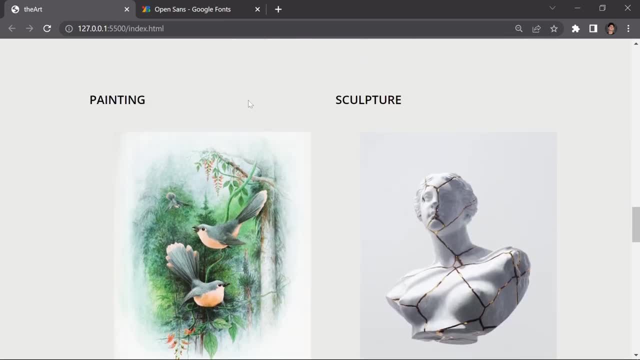 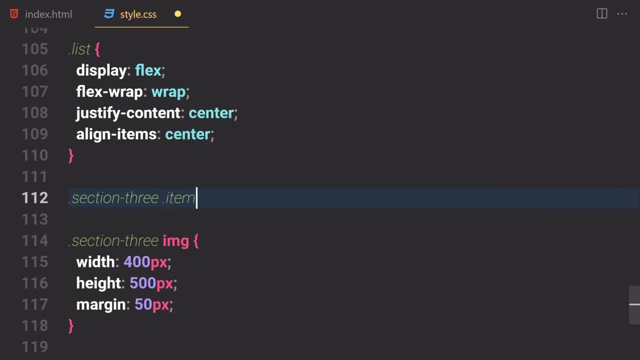 and you know what, these texts are looking a bit weird. so let's just take care of that. so what do we have to do? let's just select. or a section three. we gotta select our item and we want to select all of that edge. so we have this item, then we have our heading, then we have another. 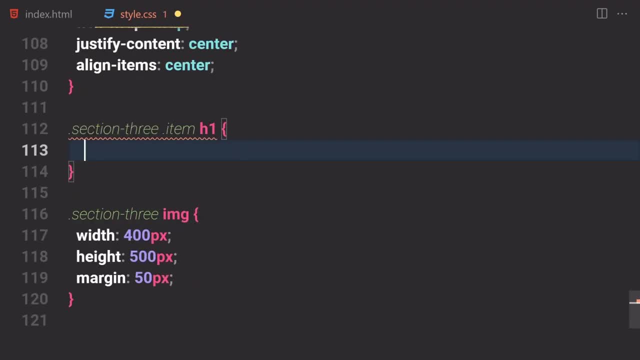 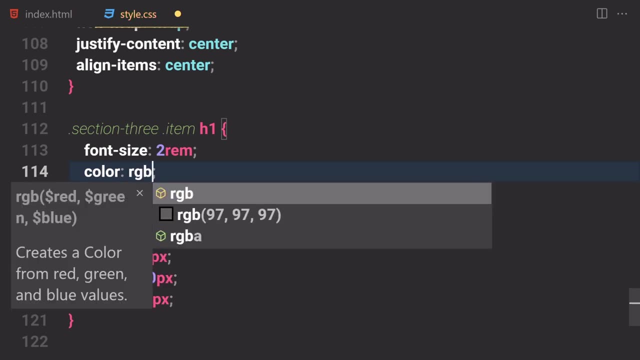 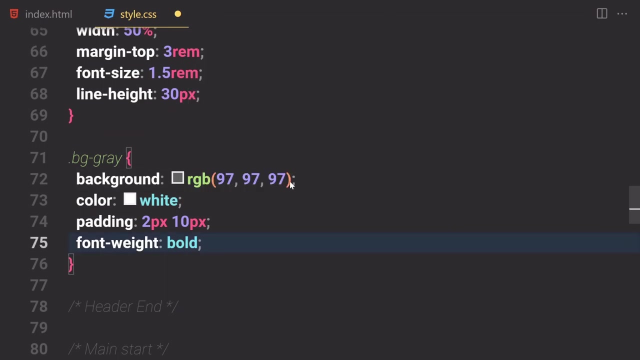 item and it's heading and so on and so forth. so now we selected that. now let's just increase the font size to be like 2 rem, and i'm going to give a color of like rgb, of that kind of 53 color where- and it's heading. so now let's just set the color for that and then we have our. that will give me. 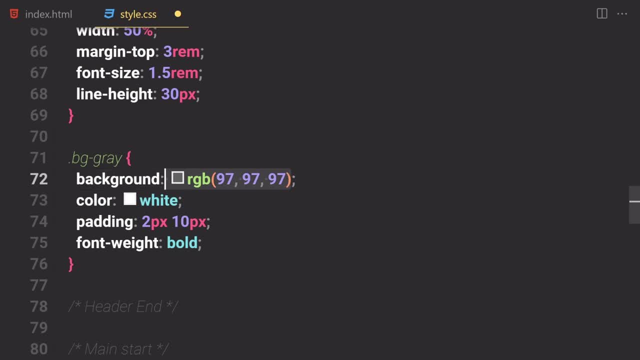 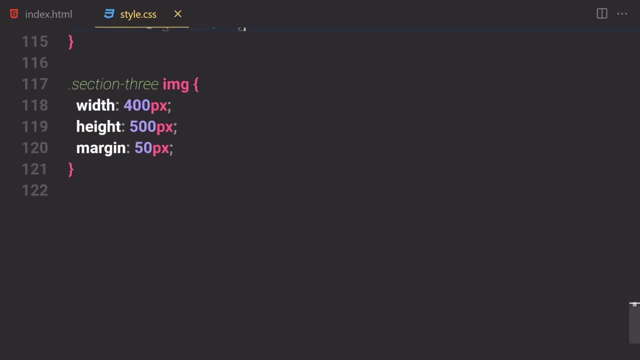 it will give me a little bit of color that i don't want to change. so i'm just going to do something like we want to change the color. so i'm just going to do something like. i didn't like that. i'm going to copy this from here. let's just call: oh, my goodness, let's just copy it manually. 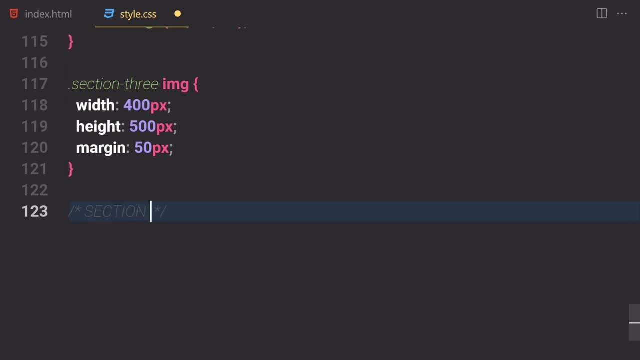 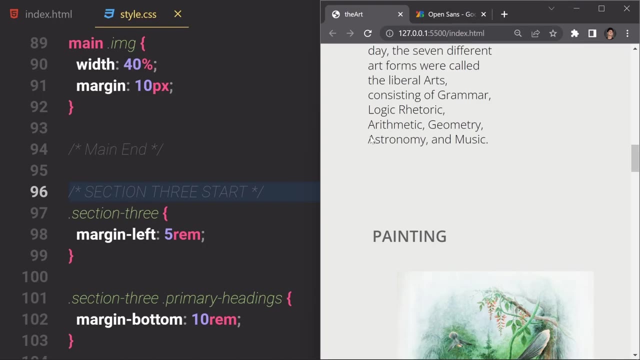 by using our keyboard. it will not allow me to use my mouse. i'm going to just use my mouse in here, past it. so we're not just changing the color of that heading, and that's awesome. so we are also done. and yeah, this is also responsive. but we can take care of that later if you want to. 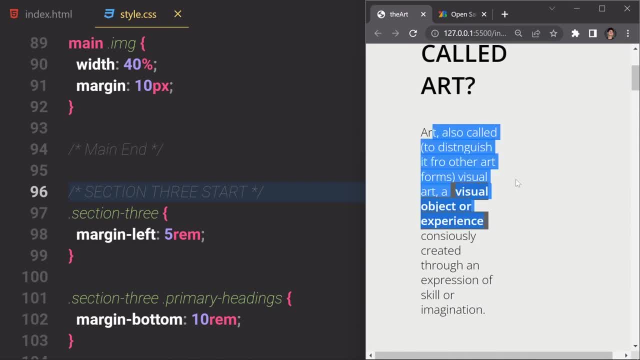 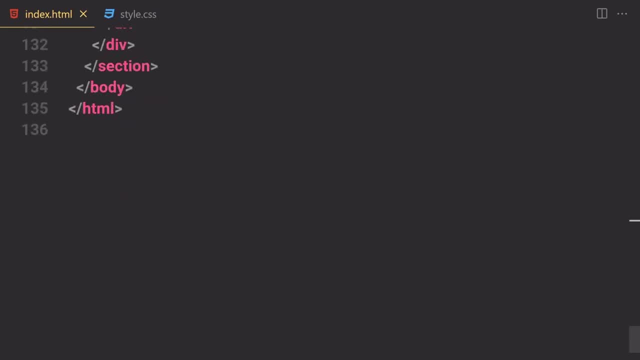 but it's already responsive, but you should have to take care of these headings and stuff anyways. so we are now totally done with section three. now let's just work on our folder area. so if you want to work with the folder area first of all- and let me just write a comment for myself- 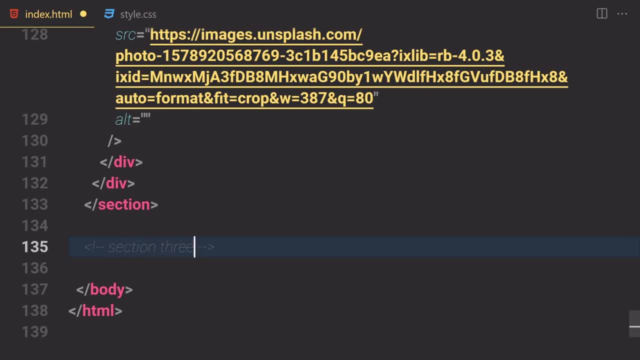 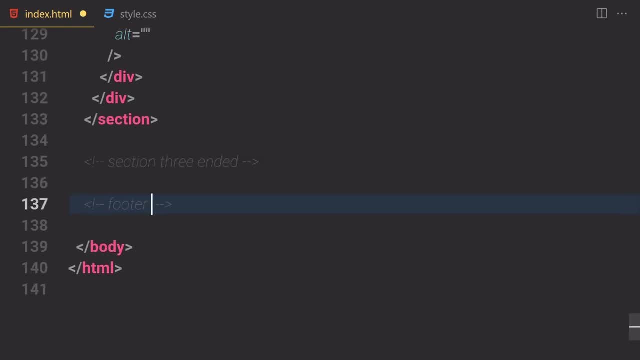 like: um, section three ended, or section three and whatever you want to call it. now let's just start working on our folder area. for start, i'm going to just write like a folder opening and closing tag. now let's just write a logo, uh, logo, oh my goodness, logo- container inside that folder and write h1. 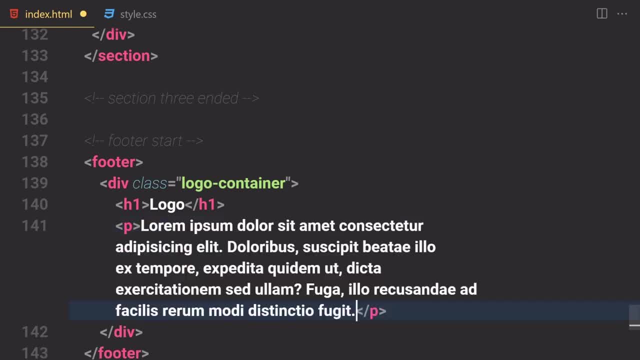 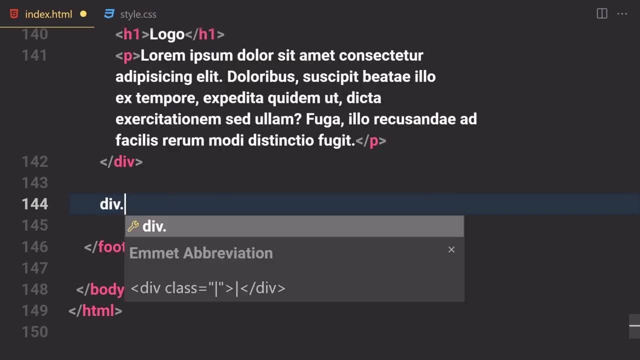 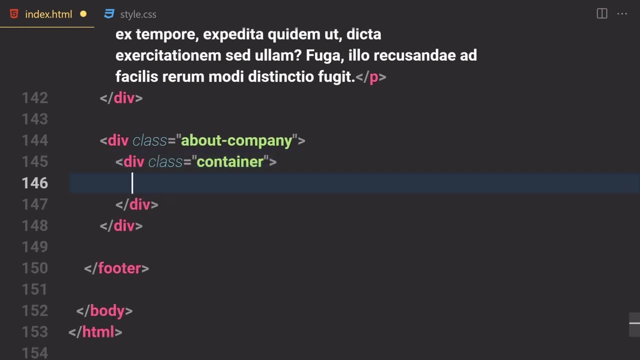 with the name of logo and write lorem and just write lorem. okay, so then, outside from this div, what do we have to do? let's just write our div with the class of about company. it's not a company, but you know what. we'll just go with that. so let's just create our container and inside this container we are going to be. 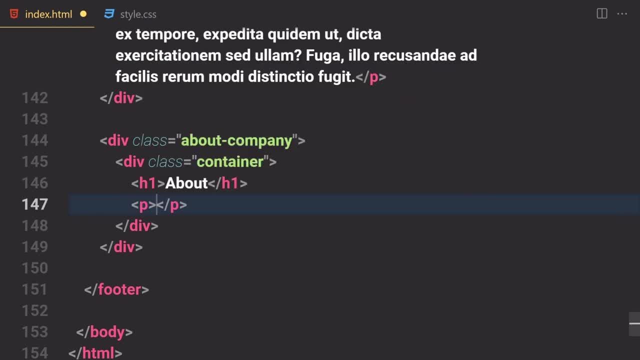 writing h1 with about, then paragraph with um, i don't know, on news and blog would be blog would be fine. uh, yeah, let's just create a new paragraph, the class of, not class, but a features text, and then we have or about us. okay, so we just have that section. let's just duplicate that a few times you. 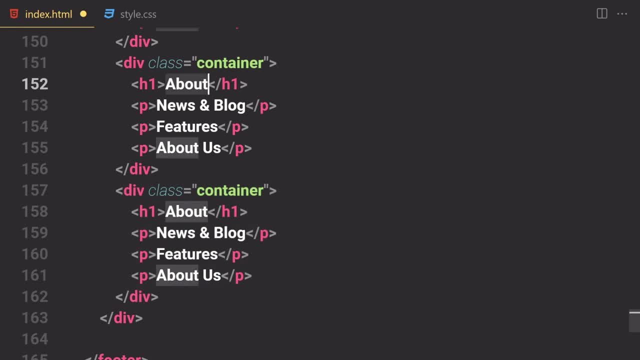 know what? i'm going to duplicate that three times now. let's just change this headings from it. so i'm going to write a company company, select that and write how we work- uh, we work, question mark, and let's okay. so i'll leave this uh feature, you know. 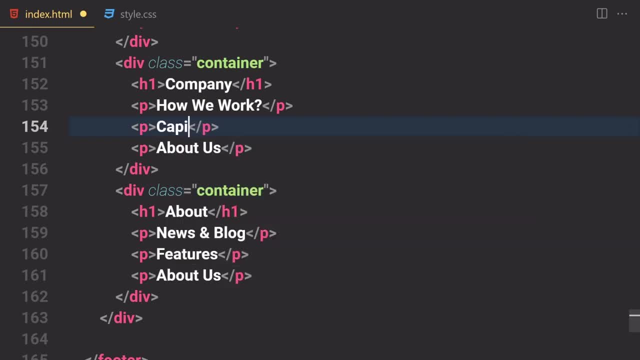 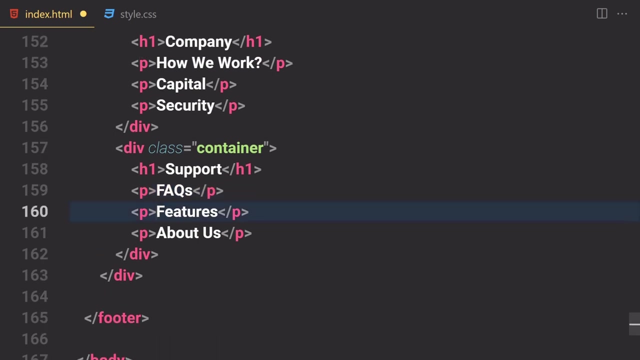 i'm going to change that to like capital, uh, capital. and also let's just remove that to security, and this one will be now support, and we have a faqs like so, or you know, i'm going to remove that comma from there and this is how it. 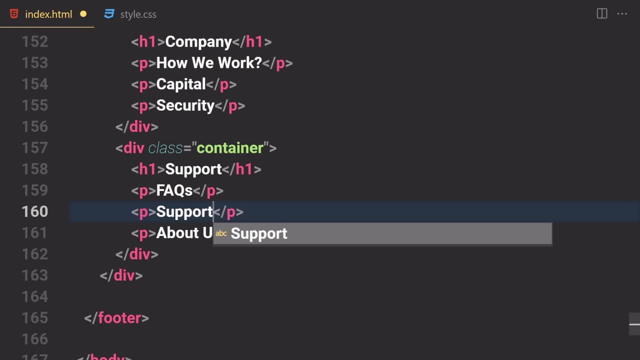 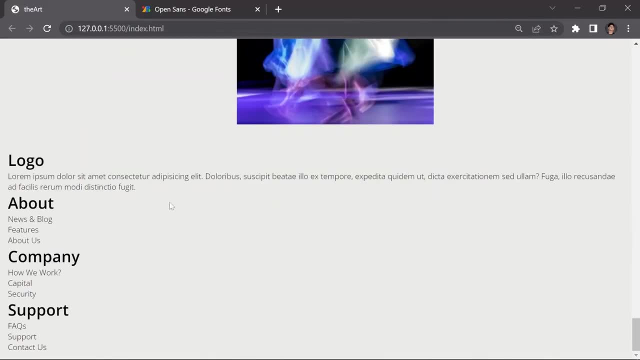 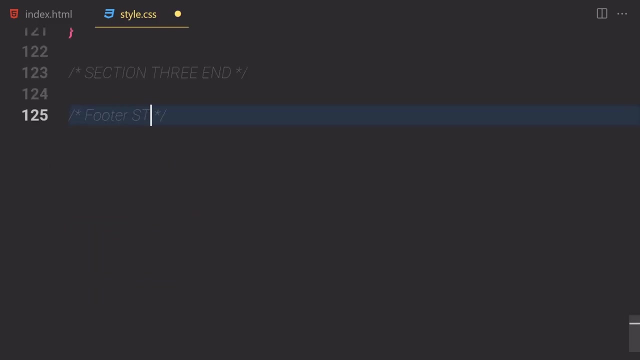 looks like, and now let's just write or support in here and then let's just write: contact us. so if you save our file, and this is how our folder will look like right now, anyway. so now let's get into our styling. and now let's just style that a bit. i'm going to write a folder: start st. 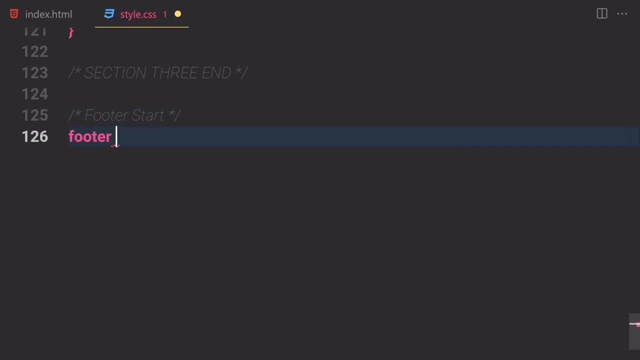 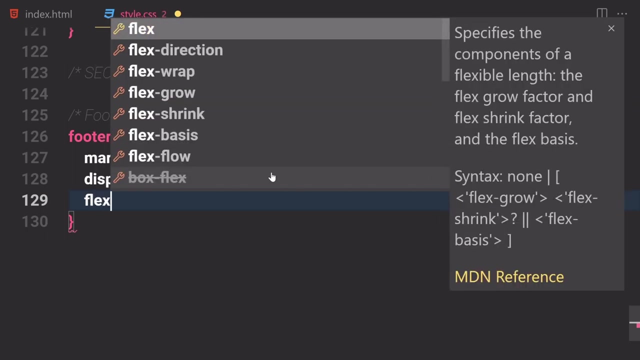 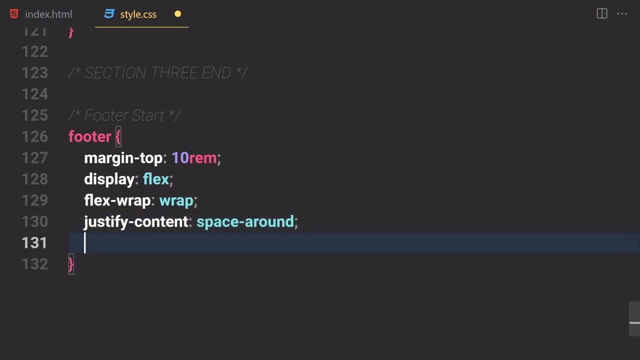 a rt? yep, let's start. so let's just get our footer area right here. i'm going to give a margin top of like 10. ram and display will be flex because we want everything to wrap up, so for that we are going to be using a flex wrap of wrap. justify counter will be space around in this case, and 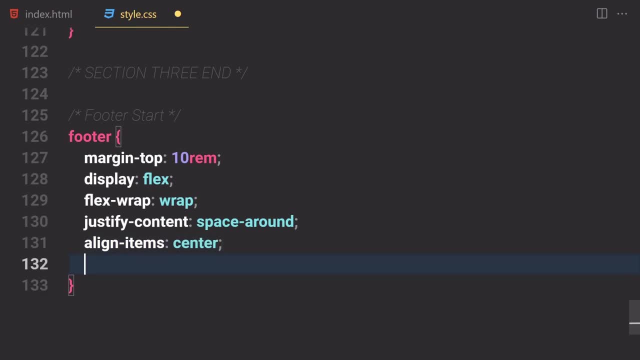 i'm going to also provide aligned items to be center. okay, so give my height of 100 vh. in this case, i'm going to bring that to the top. and now let's just write a color to be like totally white, and here we are going to be using a background color of like i don't know- rgb of 144. 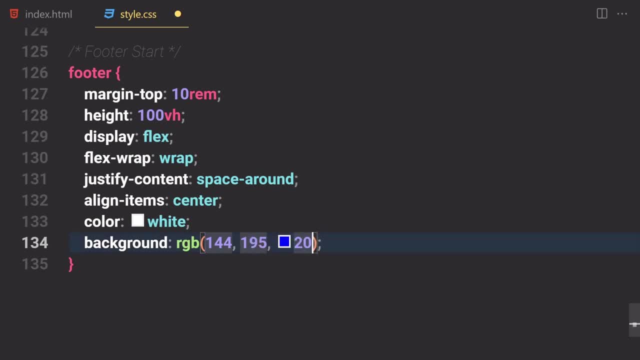 then 195 and 200 would be fine. yep, and now let's just. uh, you already gave my heart of you know what i'm going to change the height to be like: instead of 100, so i'm going to just change that to 50 vh. 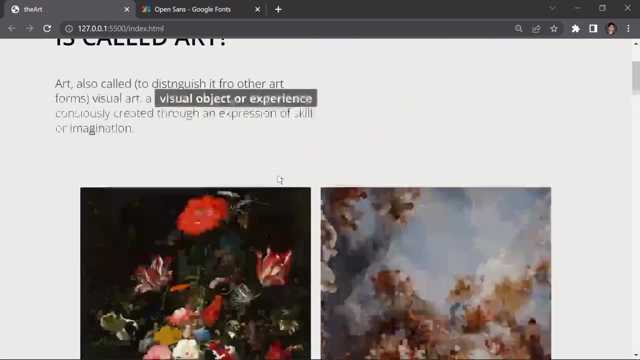 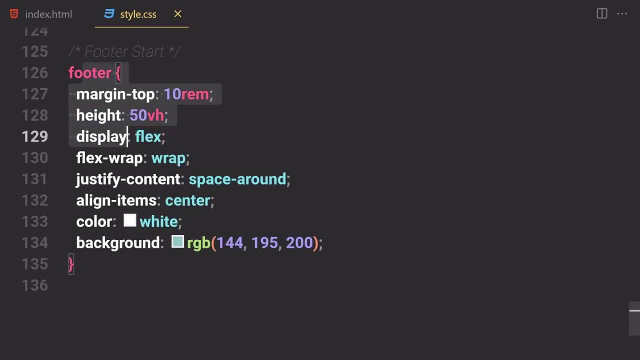 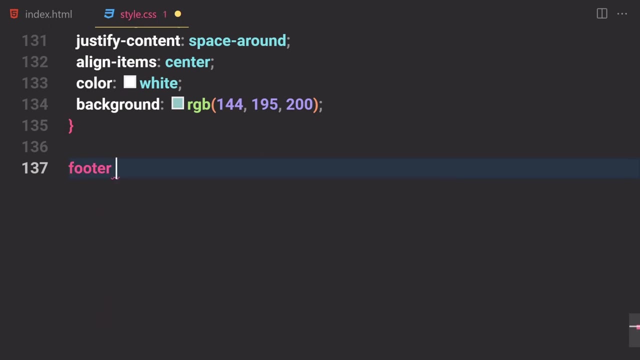 and this is how currently it looks like. and, yes, something is wrong, something is not working the way i expect it to work, but we will figure it out just in a second anyway. so this is the four area. and now what else do we have to do? uh, we have to start working on our photo logo. so let's just select our folder and 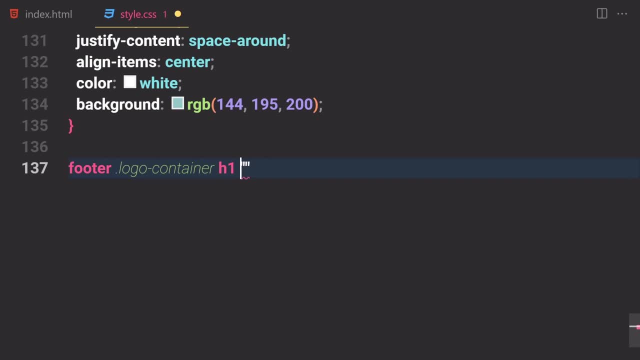 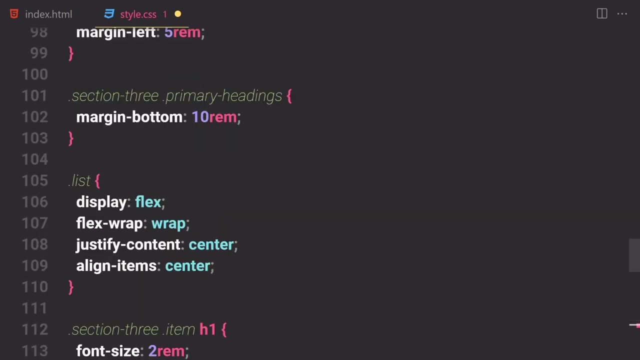 then logo container and you want to select our h1 from there. so let's just provide a font size of four rams and font family will be there. uh, okay, so we didn't have any, so i'm going to use that font family. real quick, i'm going to font that. 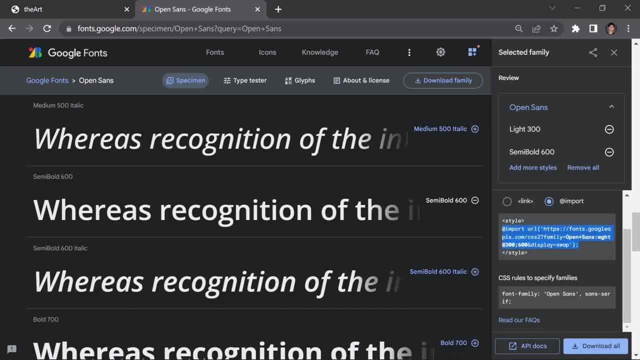 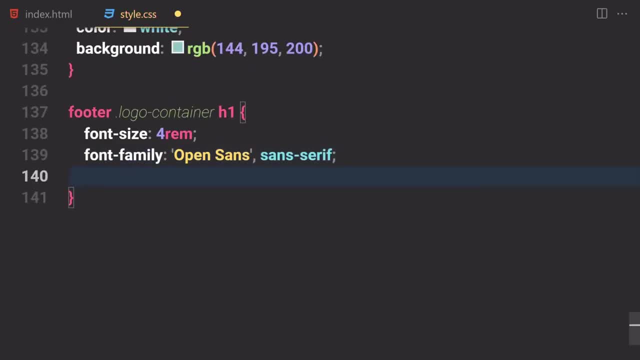 font family. and yeah, this is their open sense font family. i'm going to copy there and i'm going to paste it right here, that open sense kind of a font and now let's just use- or you know, we can also go with a sensor if you want to. so i'm going to decide margin bottom. 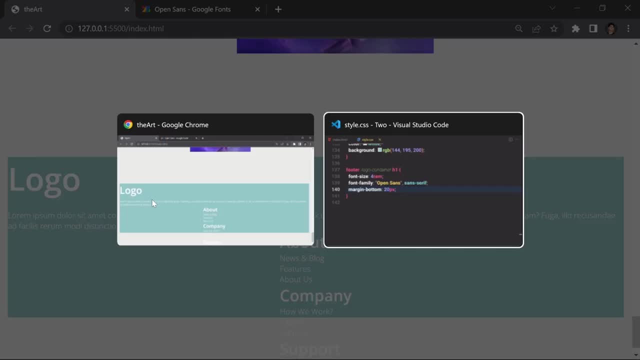 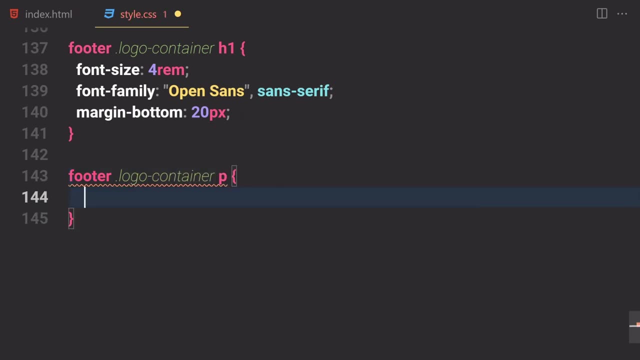 of 20 pixel and this is going to be aired for the logo. and now let's just select or folder, uh logo, a logo container and paragraph inside the logo container. you're going to giving a max width of like 400 pixel and farm family will be now set to sensor line height. i'm 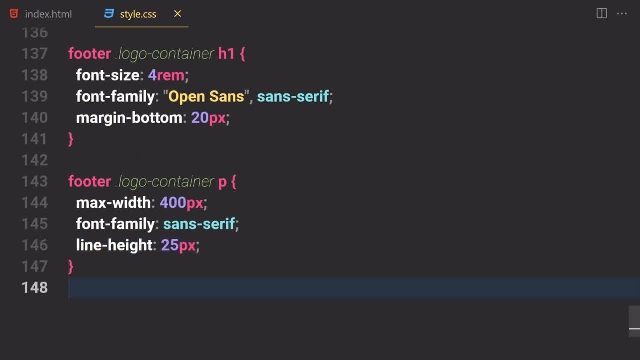 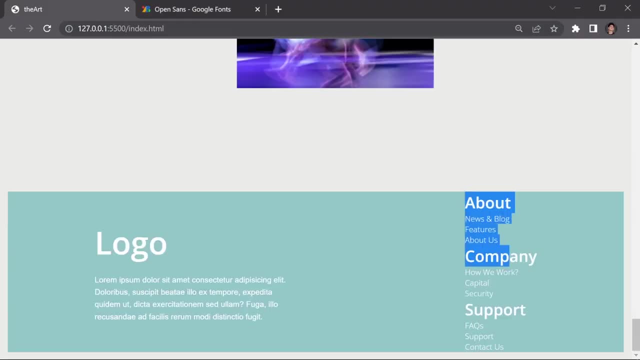 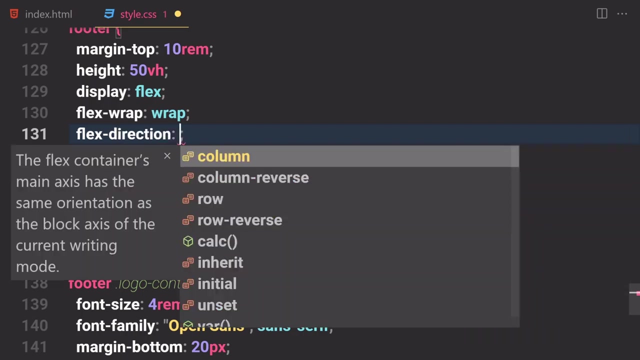 going to provide like 25 pixels. you have a logo container. do we have a logo container? yep, we do have a logo container right there and, yeah, this is looking better, but these are looking awful. i'm going to also change the direction of our flex box, so flex direction to be colon. so if you 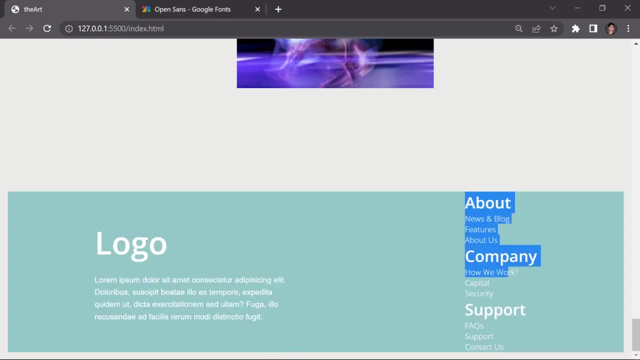 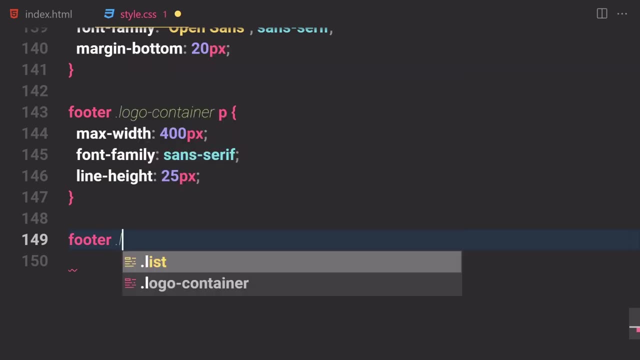 set that to column and, yep, nothing will happen in this case, so you got to do something about there, all right, so now let's just select our footer and then let's select our logo container. not logo container, but just about company which. oh my goodness, it is about company which is this: 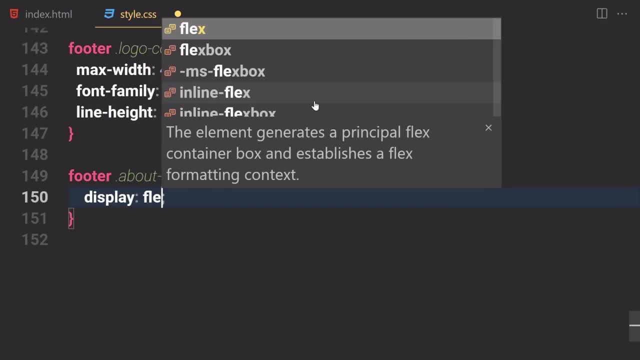 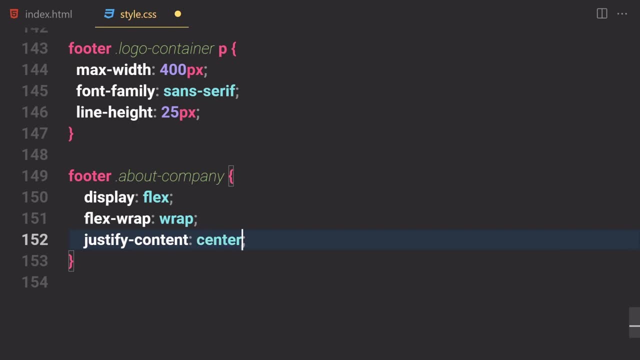 one right here. okay, so let's just write a display on flex on there and flex wrap will be now set to no wrap. not no wrap, but just wrap. justify company. content will be now set to center: align items. items will be now set to center as well, and i'm 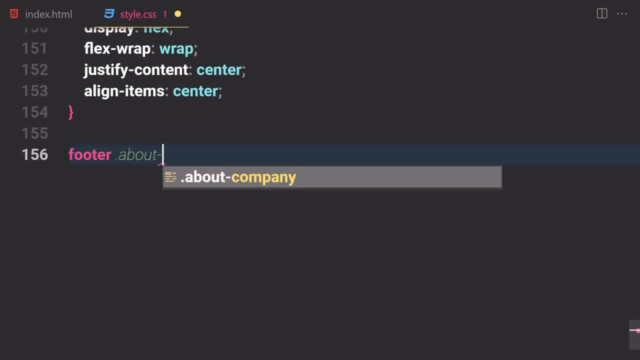 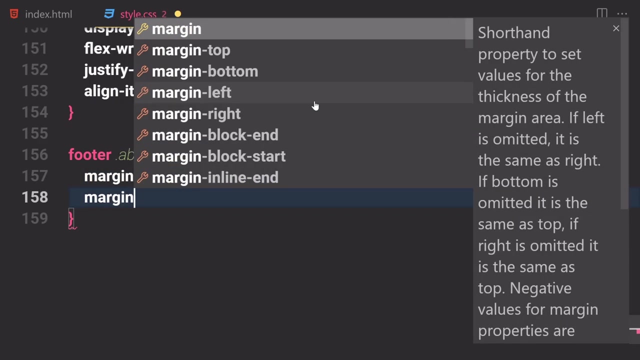 going to also select my footer area from there. and now let's just select our about company and select that container. uh, oh my goodness, can container like so and provide a margin to the right, maybe 40 pixel, and margin to the top will be 20? uh, margin top of 20 pixels. so if you save, 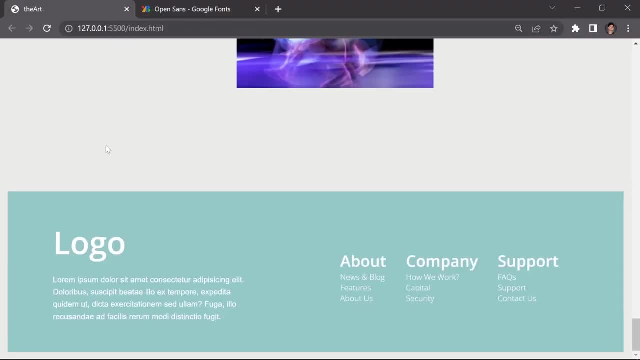 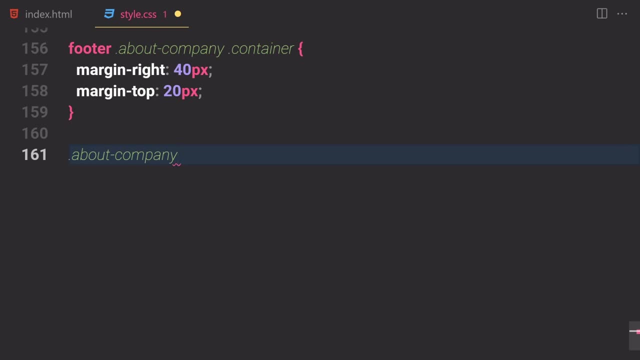 there and these are looking better, but we have a huge problem. so if we save which we need to solve, let's just type these and then we will take care of there just in a second. let's just select for about company and select for container, let's select heading, and i'm going to give a margin of 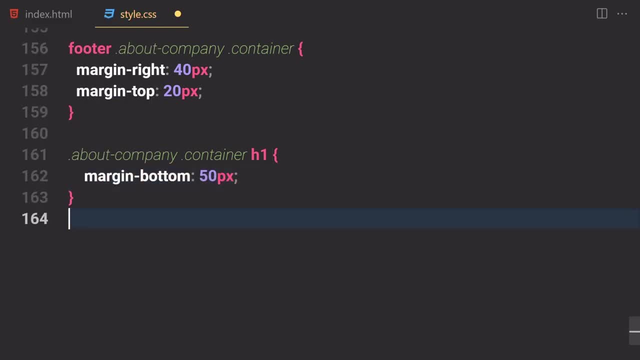 bottom of 50 pixel will be fine. let's just select or about company, and let's select our container and paragraph. and here i'm going to just write a font, family of sand, serif and margin bottom and second content. but now let's just keep doing this. let's reduce thatрен and there will be little or bridge. so i'm just going to delete this, since none's useful. but let's fix that simple now. 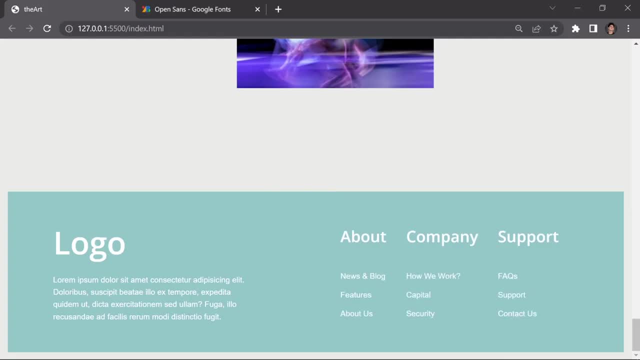 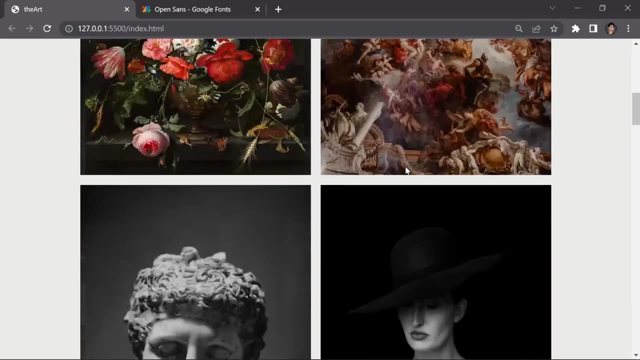 bottom will be 20 pixels if you save our file, and this is how it looks like it's looking better. but uh, you know what? we have a huge problem why it's not giving us that background color. i guess we forgot that in the first place. so we have everything we need. we have. 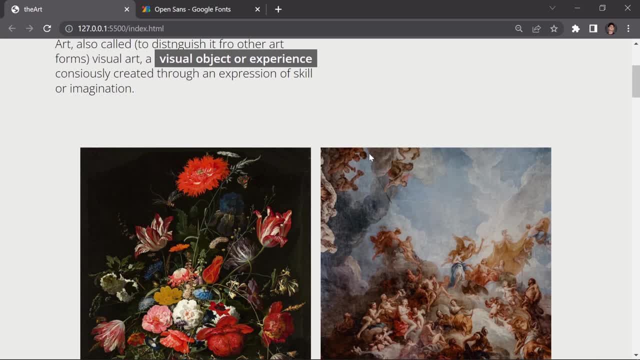 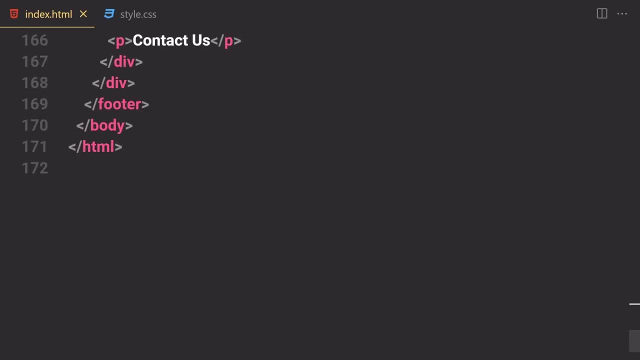 html. we have ul li burgers, we have everything, but something is not right. okay, i just remembered that we forgot to include that closing tag of the div. so now, let's just do that real quick. so if you save that, all right. so let's just see, we have our section wrapper, our wrapper container to be. 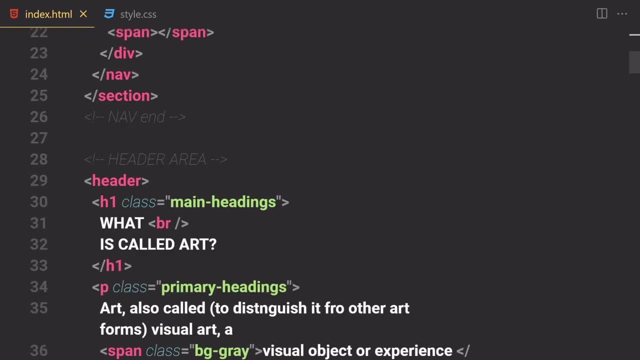 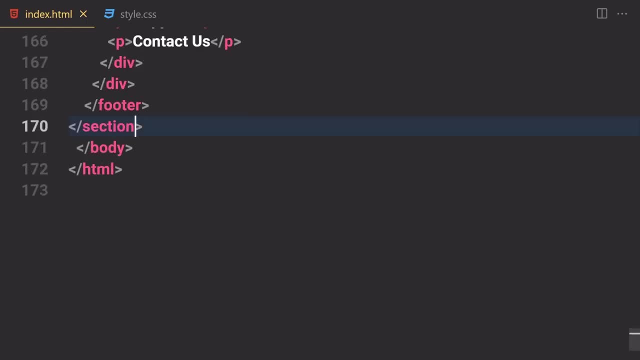 precise and where did i close? okay, so we have a section at the end. we don't have any divs. let's just close this section right here. see if you save that right now. okay, so nothing is happening and that's a huge pain. so i'm going to zoom more. 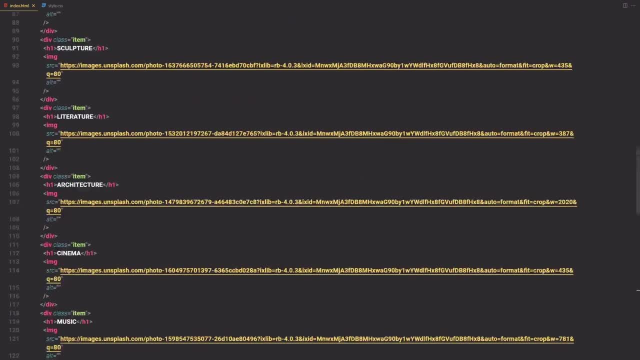 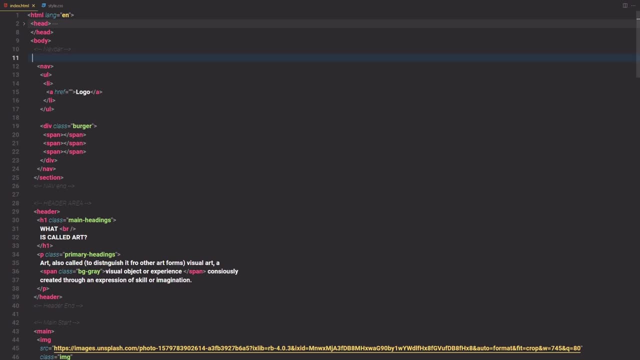 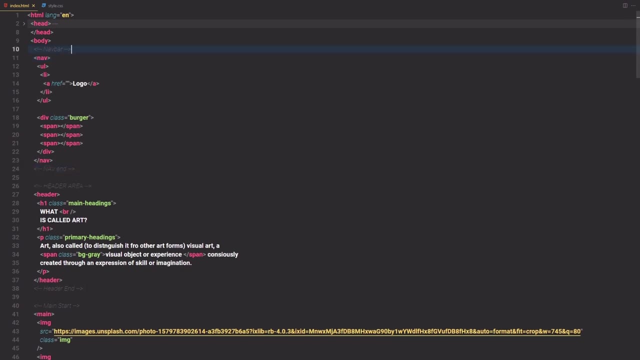 a bit a lot so i can see the coding. so what we have, we have, or, um, section wrapper, we have a body, and then we have our section rubber. something is not right. i'm totally sure about that. yep, we did close it right here. yeah, we did close it right there. so now let's just create that section. i'm 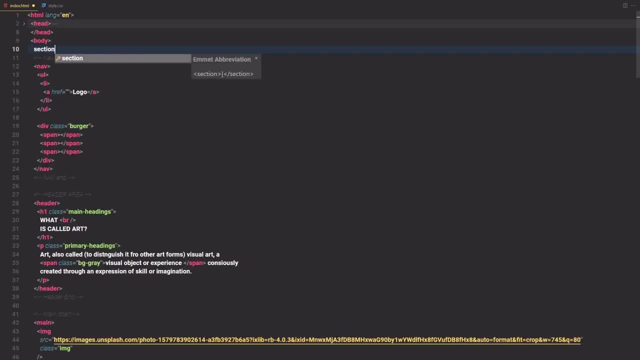 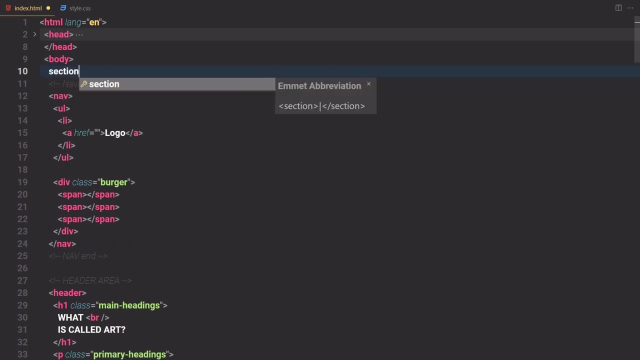 going to zoom in a bit for now. section with the class of container: wrapper. what was that? let's just undo it. so now let's just create this section one more time. or you know, i'm not going to create any section, so i'm going to just write like a wrapper container, okay, so i'm going to close that from. 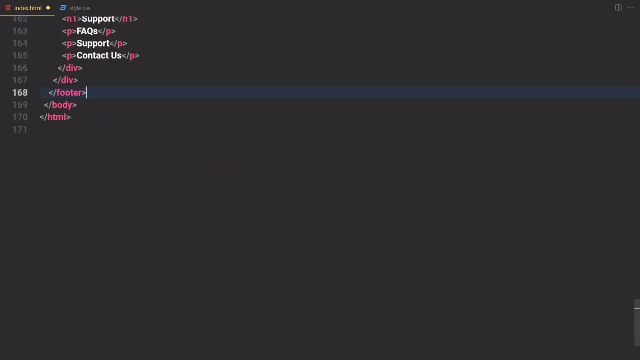 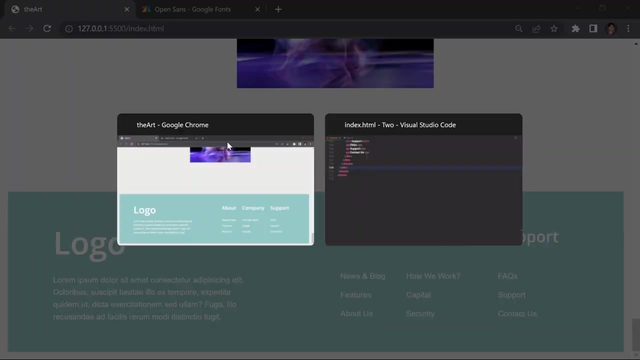 there and i'm going to paste this one right here underneath this footer. so i'm going to paste it right here and now it's looking better. but the thing still is that we didn't change the background color of it, so we have to change the background color to something else and 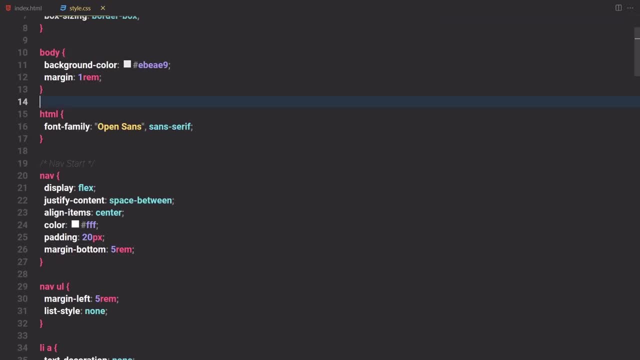 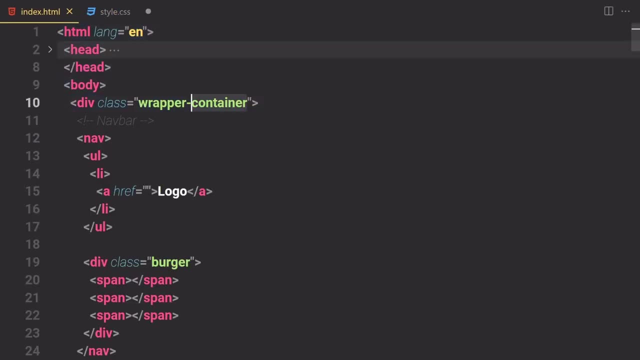 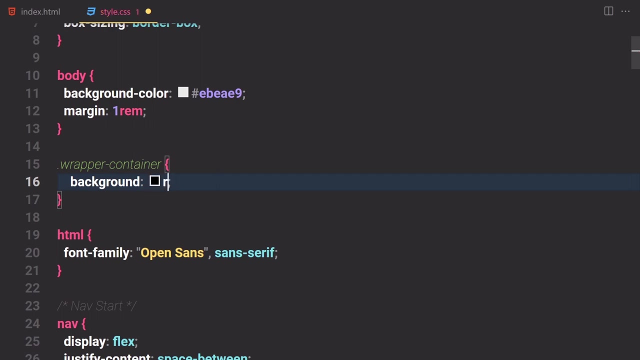 let's just select the wrapper container, which we forgot to include right here. so, uh, let's just select it. i'm going to zoom in a bit and disrupt our container, copy it and paste it. let's just change the background color of it to that background color which we just 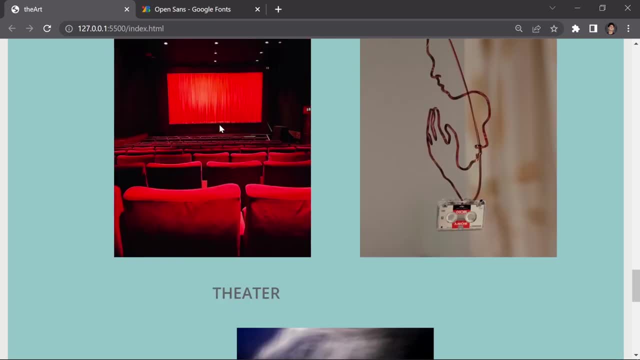 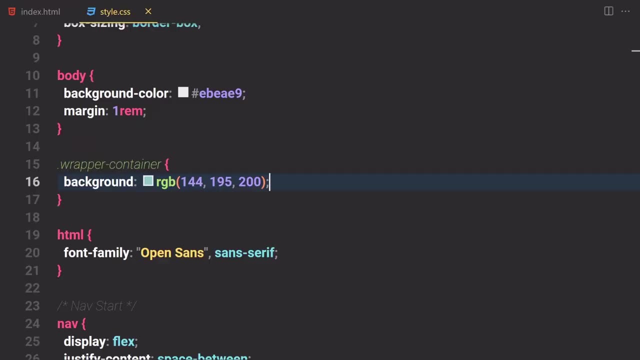 provide rgb of this one. so if you save that- and now it's looking a bit awful, we don't, we don't want that. uh, you know what? this is awful, so i'm gonna cut that from there. and what should we do? i'm gonna paste it right here and i'm gonna move it to the right side. so i'm gonna paste it right here. 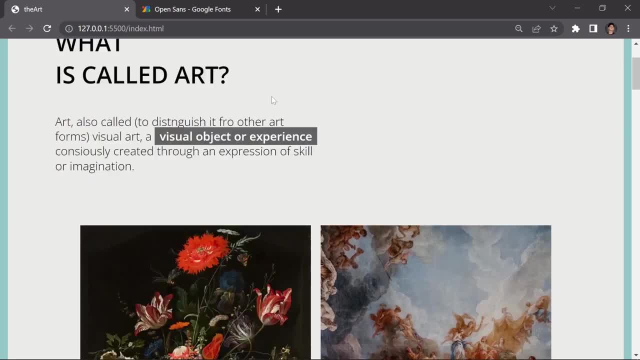 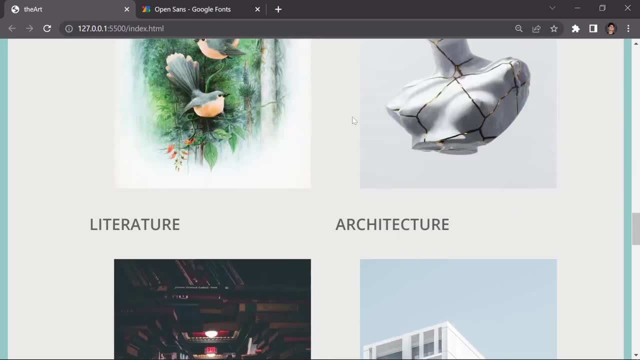 I'm going to cut that color And I'm going to paste this one right here. Yep, that's looking better. So you can provide JavaScript for that if you want to. But I guess we are totally done with our project. But the next thing which you have to take care of is that. what do we call it? 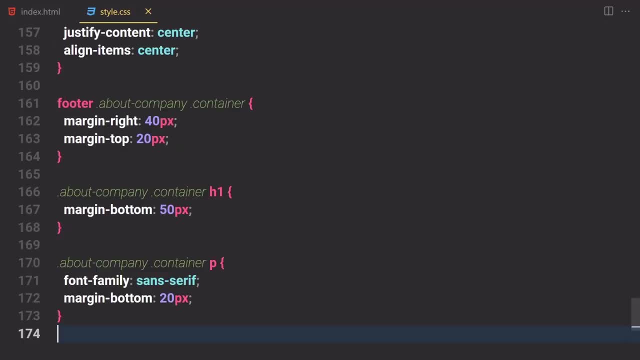 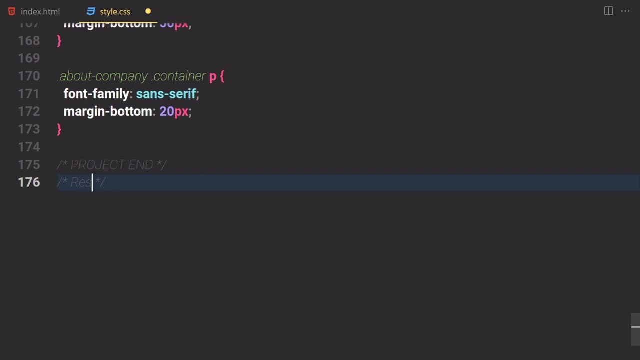 immediate queries and responsiveness. So now let's just take care of that. I'm going to go to the bottom, Yeah, I'm going to just write like project and and now let's just write response. So, yes, yeah, zoom in a bit, zoom in a bit, not out. Okay, so media, let's just create media for that. 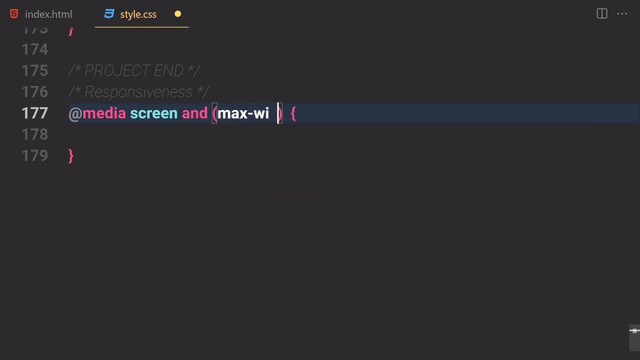 we are going to providing an N max width. width is over, like 740.. Let me just get my keyboard 700 and what? 740 pixels. So what do we have to do? we have to select our header, we have to write a main headings, select that and we have to give a width of 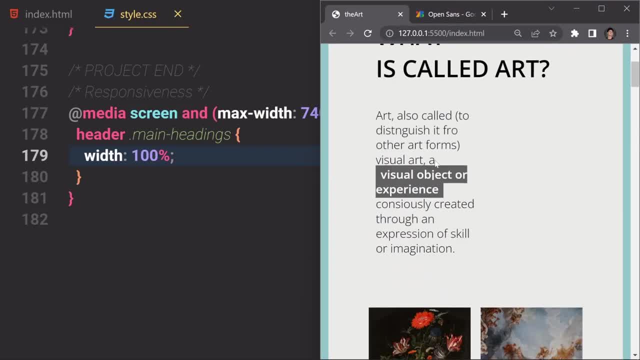 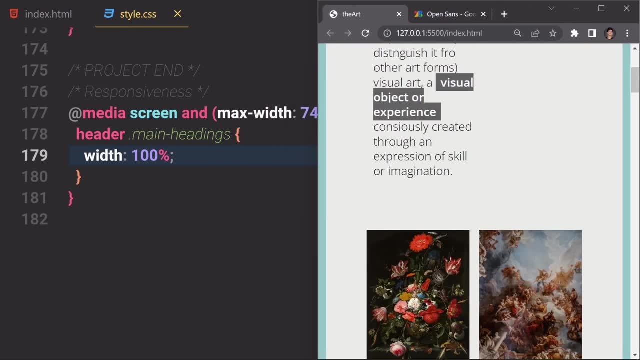 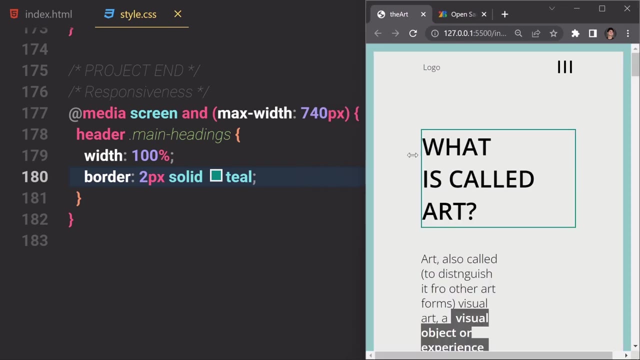 100. percent. so if you save that, let's just make it smaller so it will take a hundred percent of its space. so, okay, it's not working. let's just write a border of two pixels solid teal, okay. so it's not taking its area right here and it's taking 100 of your space. that's looking. 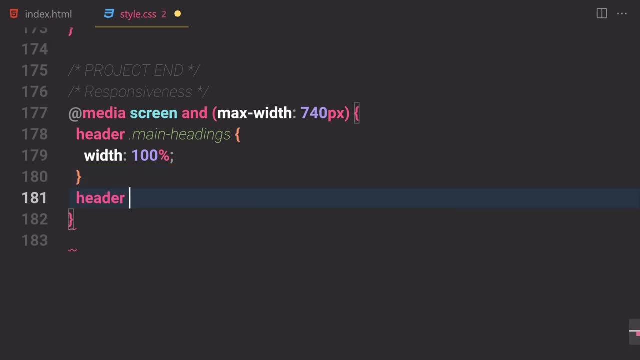 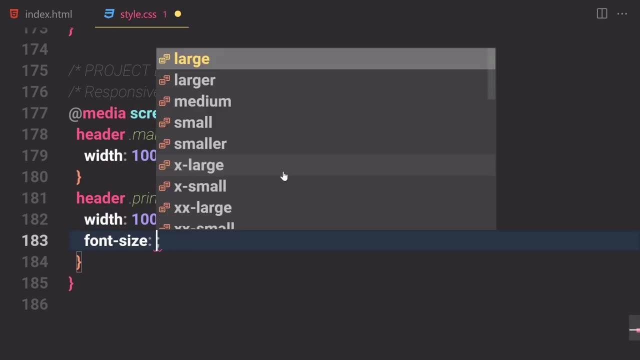 better, all right, so now let's just select our header and select our primary headings. in this case, we're going to be also changing the width to be 100 and the font size: i'm going to just change that to 1.5 for ram. so if you save that and yep, that's looking cool and everything is. 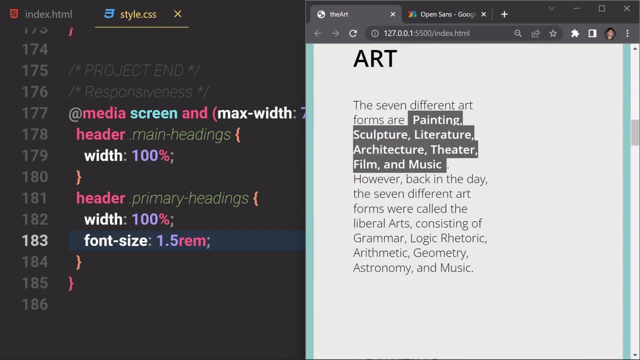 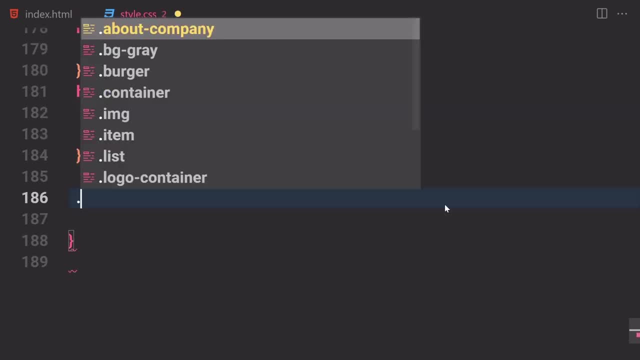 totally responsive, but now let's just take care of this area as well. so for them, what do we have to do? i'm going to just, uh, duplicate. oh you know what. let me just write a manual. then you might be complaining, but you just duplicate your code. let's just select word. section three and main headings. 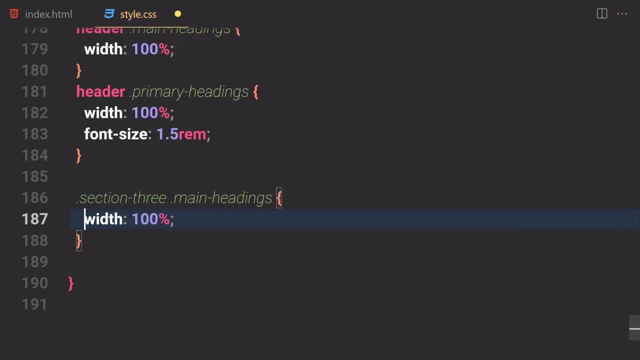 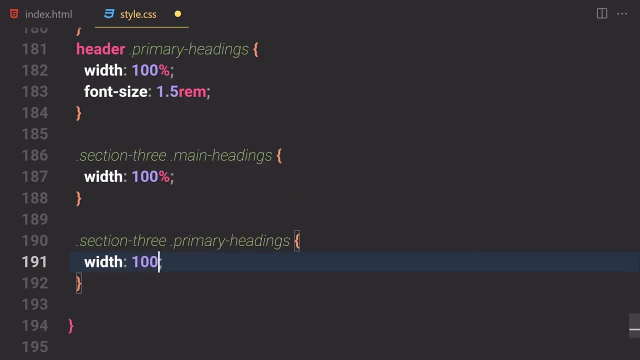 and we are going to be writing, or width of 100 in this case, and then let's select what section three of primary headings of width. let's just get 100 width, font size of 1.5 frame and finally, let's just make these images a bit smaller. so i'm 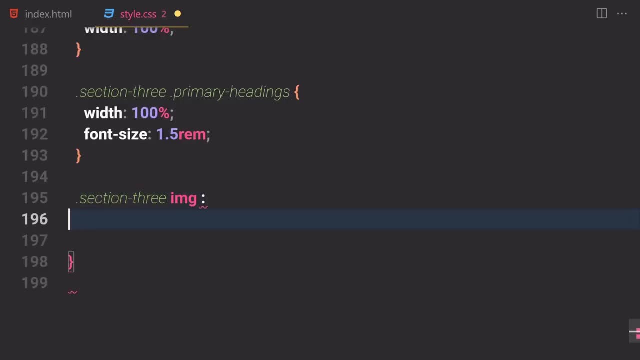 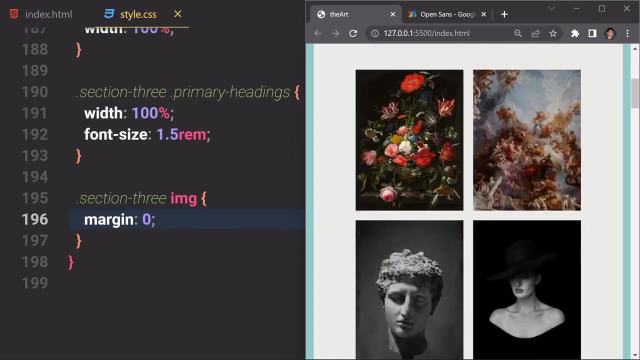 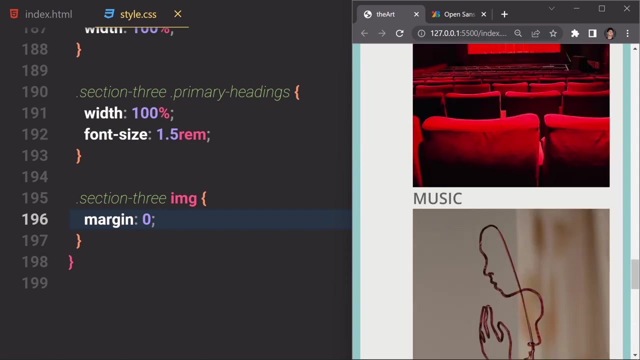 going to just select my section 3. let's just get all of the images and, uh, let's just write a margin of zero. so if you save that- and this is how word side looks like for now- it's looking totally responsive and awesome, and we are not totally done with our second project as well. so i guess 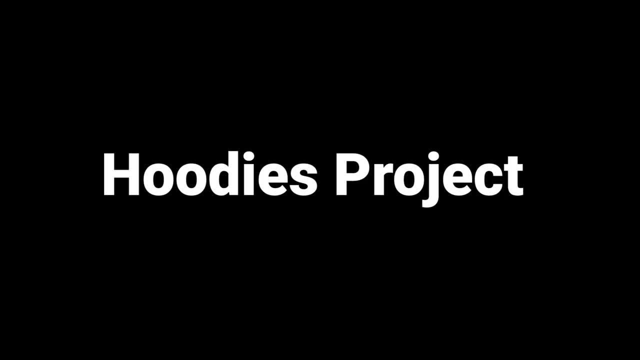 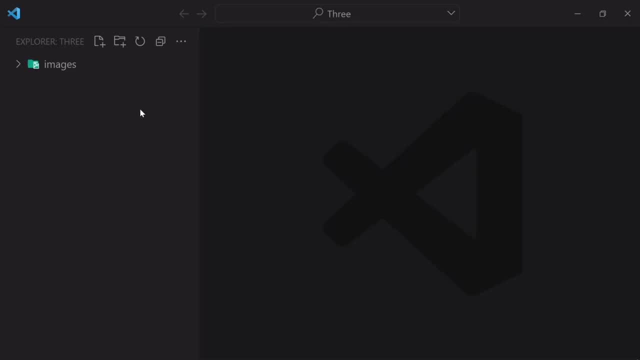 that will be it for now and i'll see you in the next project, all right, so if you want to follow along with this video, you will find a link in the description area which will bring you to my github repository and you can download all of these images from there, if you want to use these images. 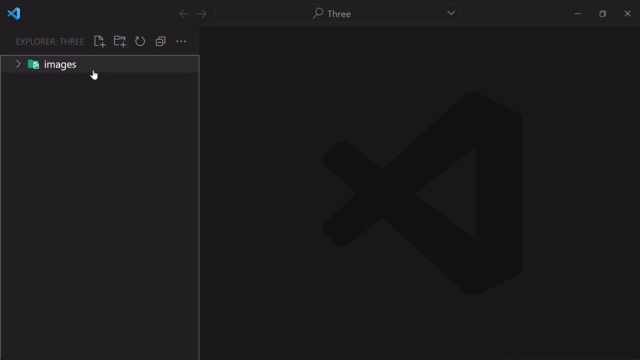 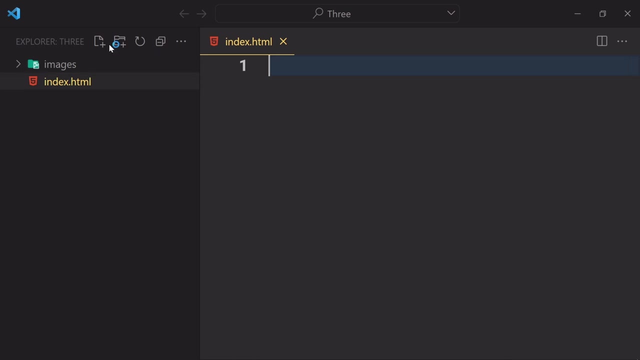 so if you want to use your own images, so feel free to do that. if you want to use my images, so you will find a link in the description below. so what do we have to do? first of all, we have to create a new file with the name of indexhtml. 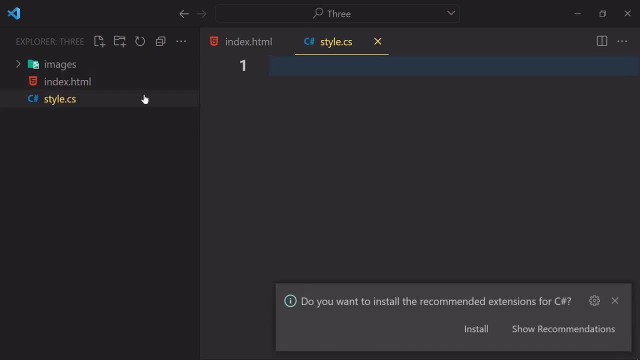 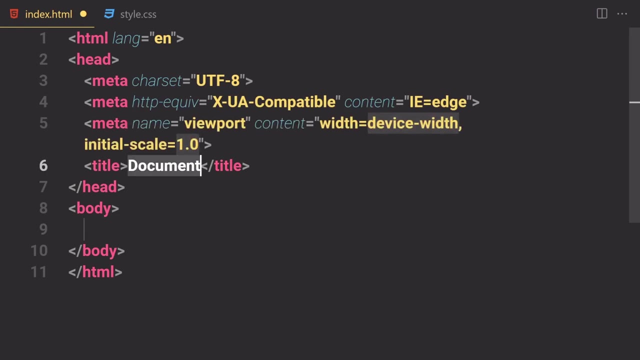 let's just create a new one with the class- not class, but the name- of stylecss. and now let's just make everything a bit bigger so we can see everything a bit clear. write a doc type html, and the name will be hoodie in this case. so collapse this hoodie from there, and you know what collapse? 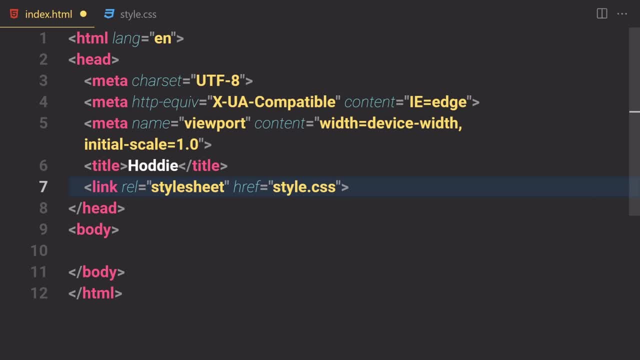 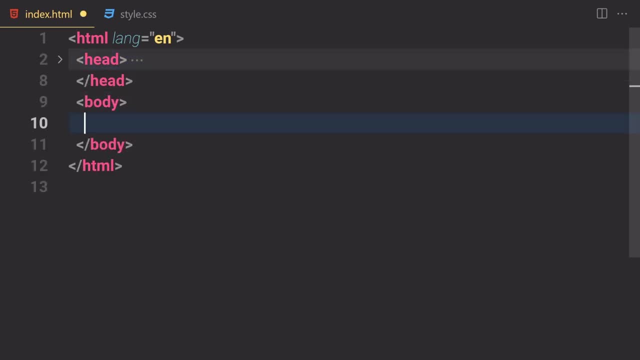 this hoodie collapse this head area, link it with our css, save our file, right click on it and open it with a live server, so that everything will be in the same way. so let's just create a new one. and now we can see everything a bit better. and we can see everything a bit better, all right, so 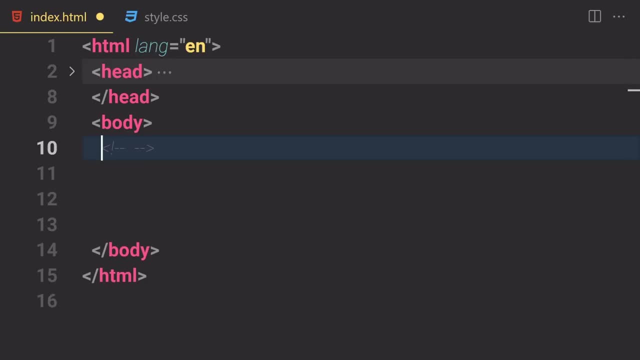 what do we have to do for our navigation? so we are going to be starting from our navigation, so i'm going to just write like a nav start, and now let's just write our navigation and inside this navigation we will have a div with the class of logo. inside this logo we will have 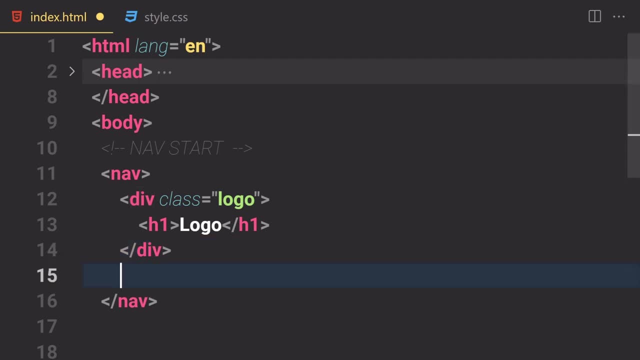 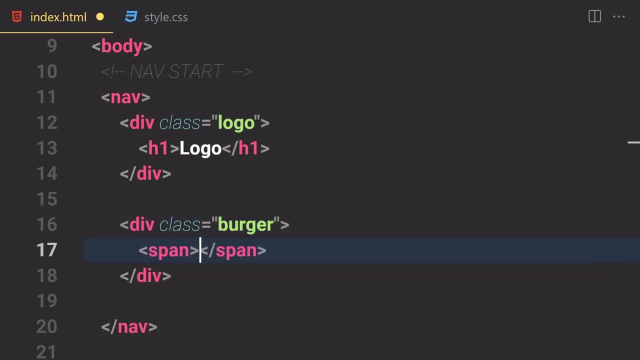 our h1 with the text off logo. so, outside from this div, what do we have to do? we are going to be creating our burger menu, so we are going to be just writing a name of burger and inside this burger we would need three spans. so if you save our file, you will just see a logo right here. but 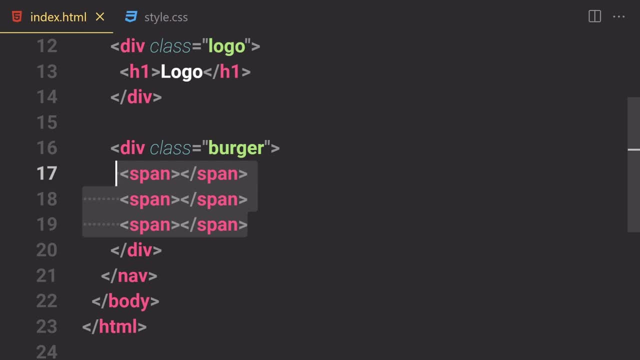 we will not see this um burger area. that's because we're going to style that and we don't have any content for that anyway. so now let's just get into our css and now let's just style that a bit. so for css, first of all, let me just write a resets for myself. so i'm going to select everything and 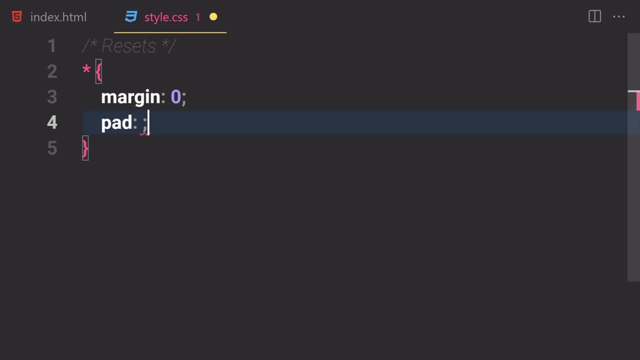 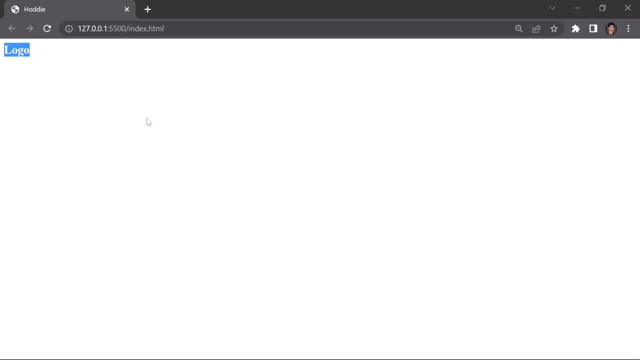 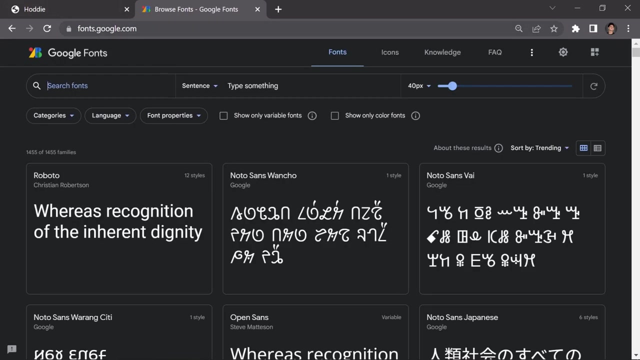 i want to just provide a margin of zero and padding- oh my goodness, not pad, but padding- will be also zero. box sizing will be set to totally border box. and now let's get into their fontsgooglecom and just grab our fonts. so for this project we would need two fonts. so i'm going 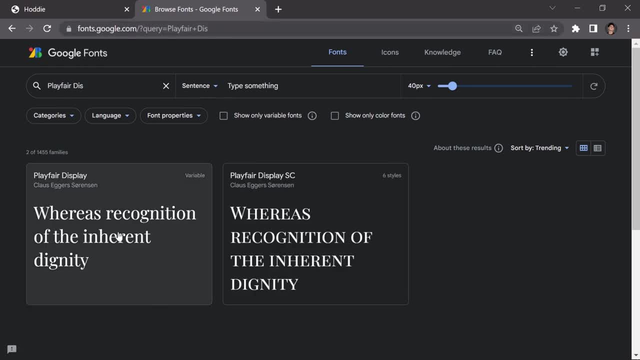 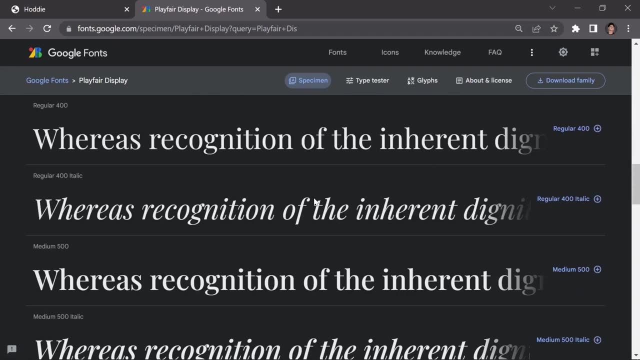 to just write play fire display or play fair display, whatever you want to call that. so i'm going to just click on this one now the other one, and we would need the font width of that. i don't know which kind of font width should we grab, and i'm going to just scroll down and i'm going to 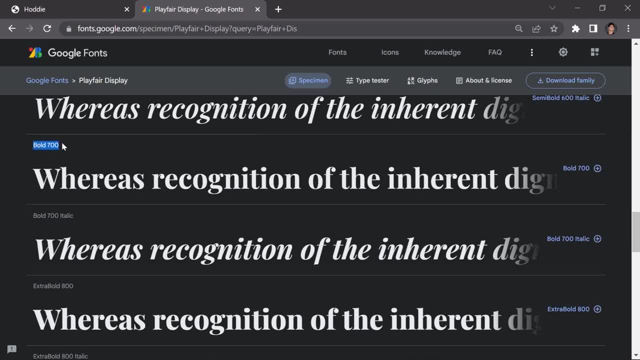 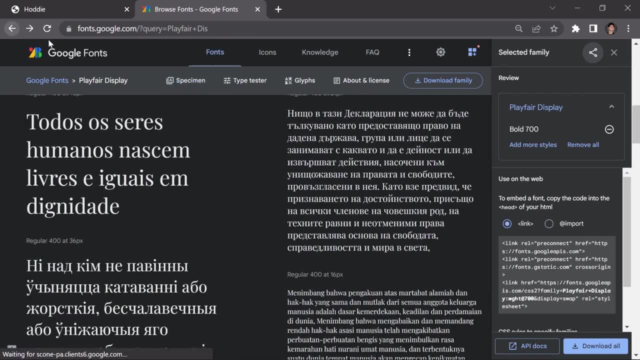 click on that 700, not italic one, but this regular 700. so i'm going to click on that one, so choose that one. and what else do we need? so we are going to be also searching for roboto one, so click on that. search for roboto font. 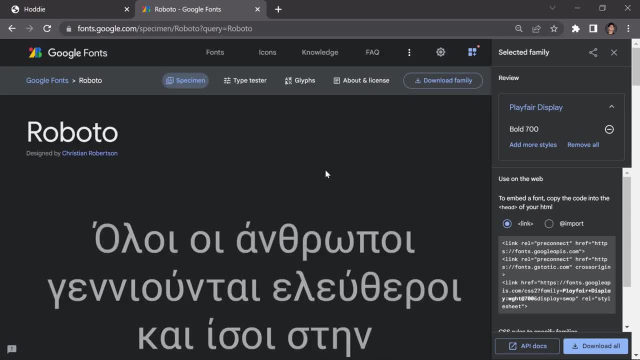 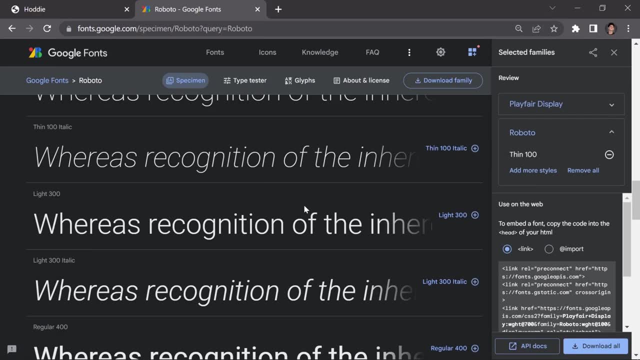 and yep, i'm going to click on this first one, and the font family which i'm going to be choosing is 100 and 300. so 100 will be the first one, the thin one, and then we have a 300 regular, not italic one. so now let's just click on this import button right here and copy this import. 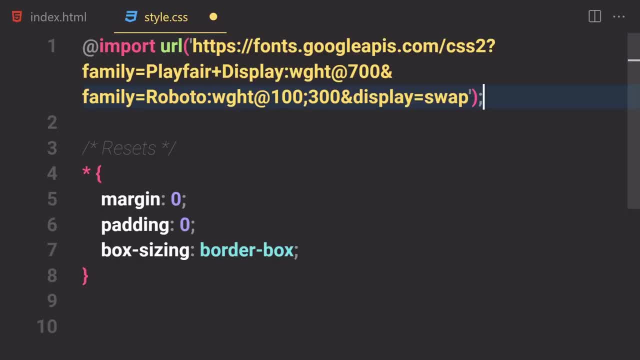 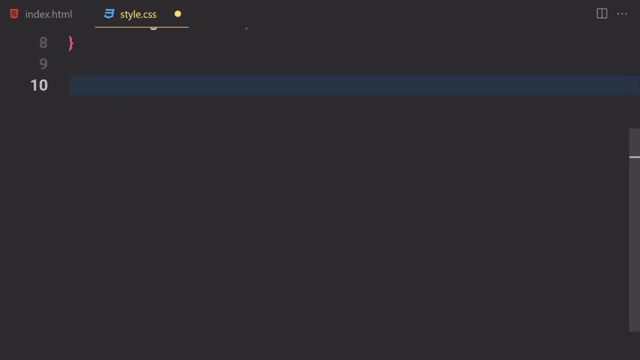 port url and paste it just past the top of this file, and we are going to be also copying these links. so let me just grab that. and you know what? let's just create a variable, real quickly, so we can store our data inside there. so i'm going to just write like a root inside this root. let's just 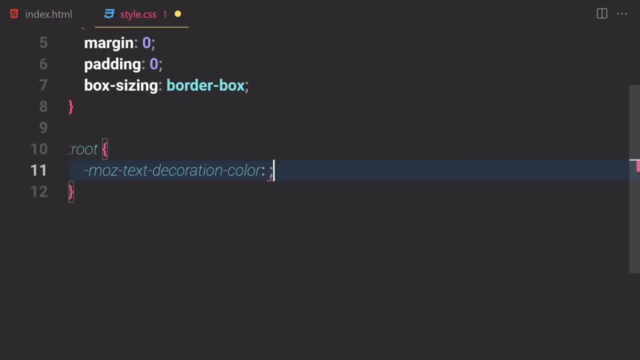 create our first variable, which will be like: uh, you know what, let's just write- or main font. so before we do that, let's just write two dashes in there and i'm gonna paste this uh link in there. let's just create a new font like primary. 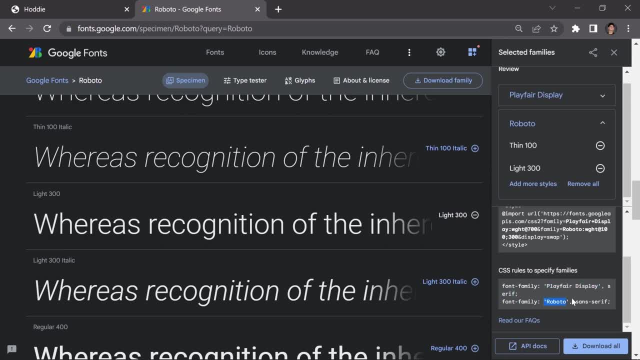 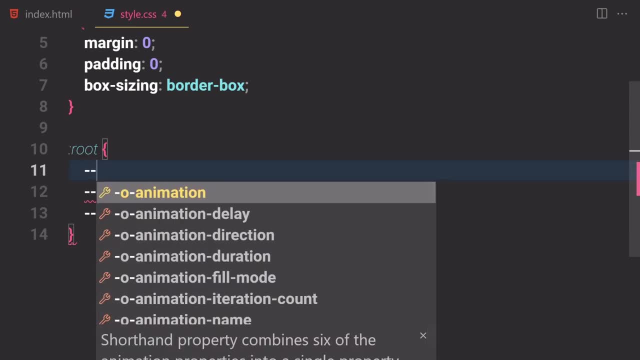 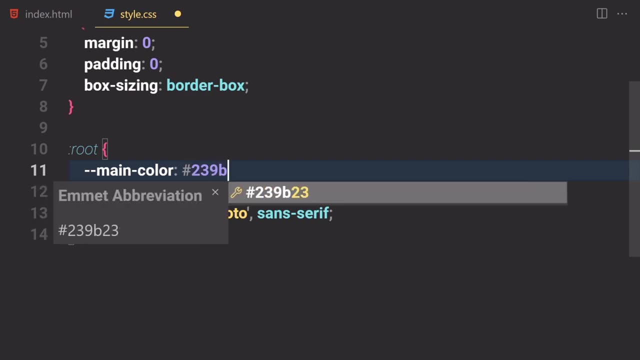 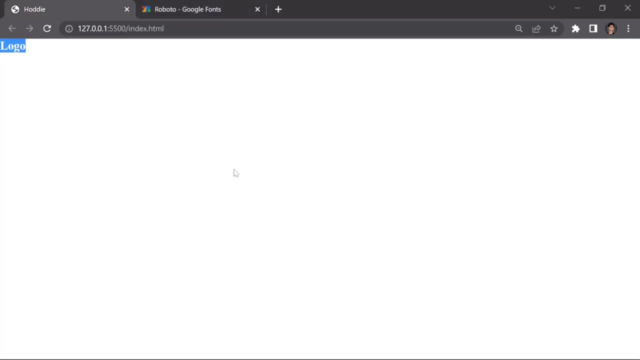 font and grab this link, which is that roboto one, and i'm going to paste it right there. and you know, i'm going to also create a class, or not a class, but a main color variable. so i'm going to write two, three, nine and b7, b7 e, okay. so i'm going to just save that and yep, you are totally good to go. 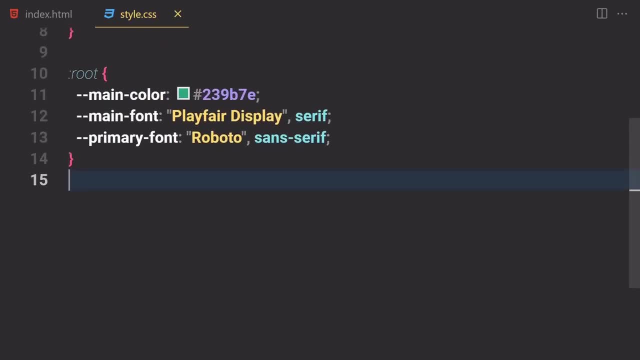 so now that was just kind of a setup. so now let's just start working on our navigation. so we are going to be writing a comment for itself like: now start, and let's start working on our navigation. so the first thing which you do is that we are going to be just writing a display of flags. 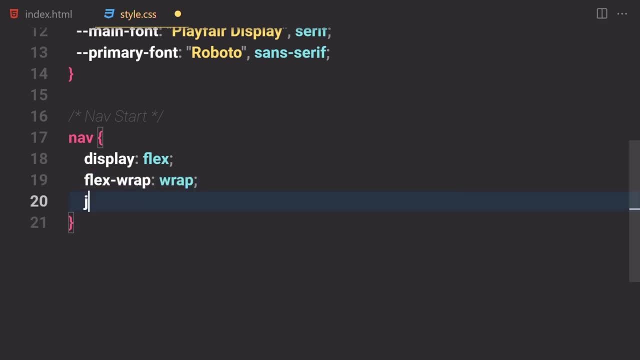 and flags. wrap will be now set to wrap and then justify. content will be now set to space between. let's just write: align. items will be now set to center and padding. i'm going to give like 20 pixel all around font family. i'm going to be using a main- not main, but primary font and then font. 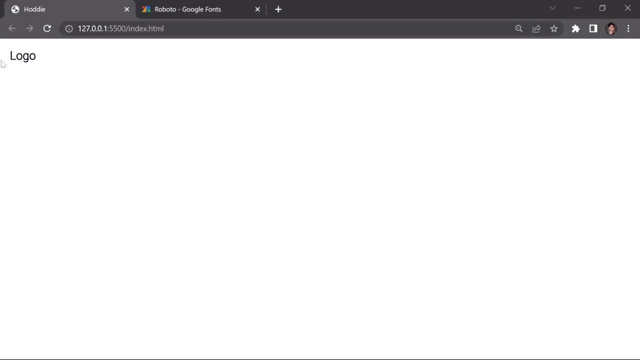 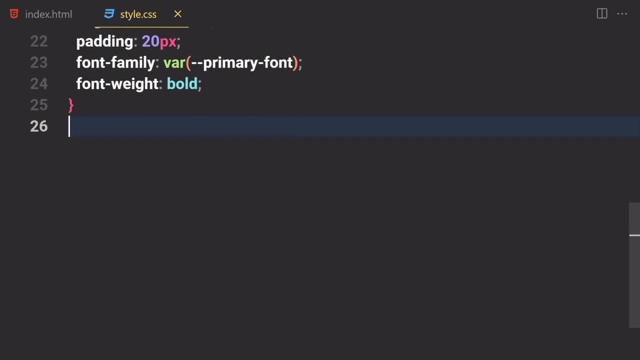 i'm going to set that to bold, so now, if you save this file, so here you can see we are now getting this logo, but we cannot see the other stuff, like burger menu and stuff like that anyways. so let's just give a little bit of margin. 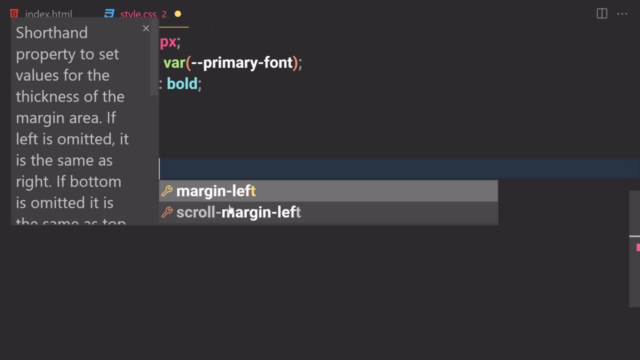 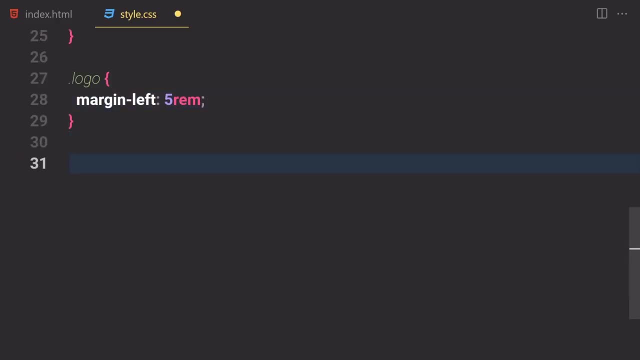 with this logo, so logo margin from the left. we are going to be providing our five frames. so if you save that- and yeah, we get a five frame of margin- now let's just start working on our burger, which is that burger right here? okay, so what do we have to do? we have to just write a display of 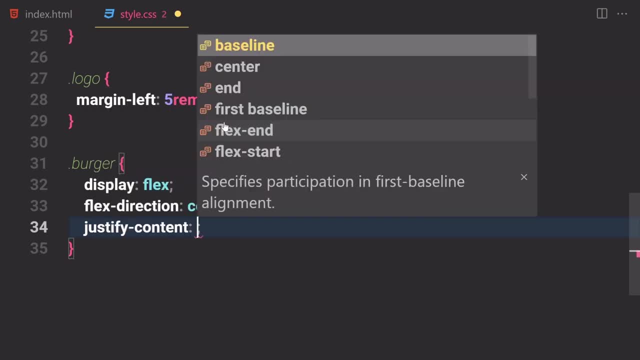 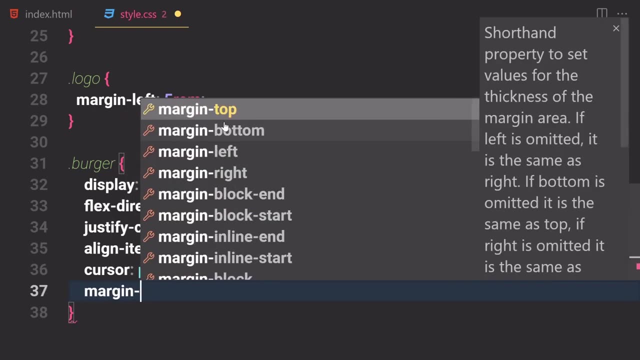 flags. flex direction will be now set to column and justify content will be now set to center. align items will be now set to center. cursor will be now set to pointer and finally, let's just give a margin to the right of five frames. so if you save that, we can still see nothing right here. 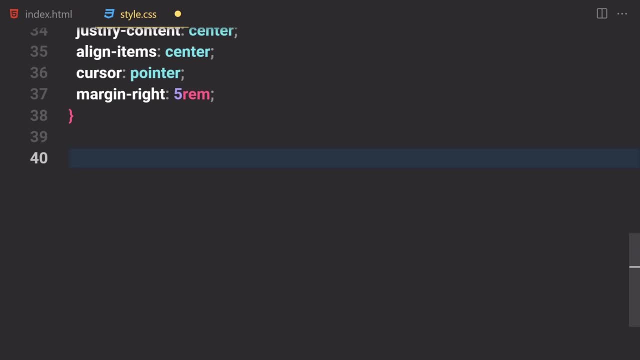 that's because we didn't select and we didn't style that spans, which is inside this burger area. so let me just get these spans real quick and i'm going to just write a span, burger and span and let's just give him a border of two pixels solid of that war which we create, that main. 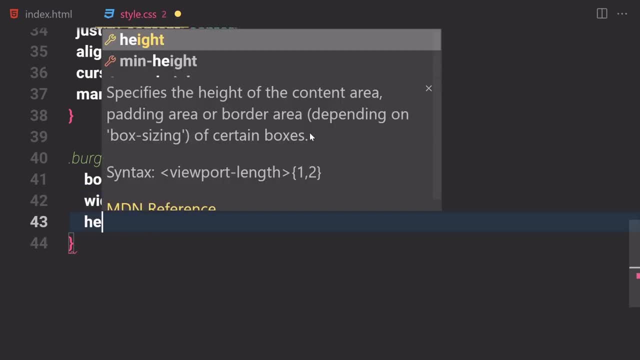 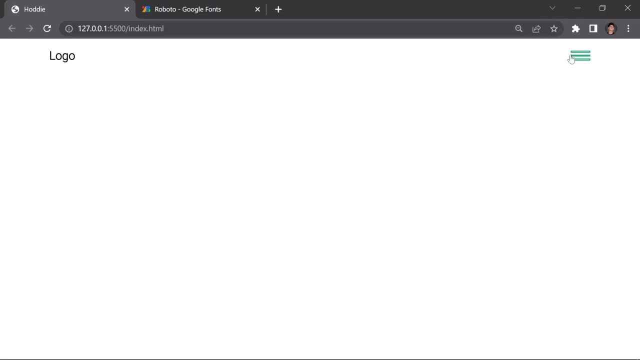 variable and let's just give him a width of like 40 pixel, height will be just one pixel, and margin: i'm going to give him like not only, but just two pixels. if you sell a file, and this is how it looks like right now, okay, so you can change that if you want to, but in my case that's looking better. 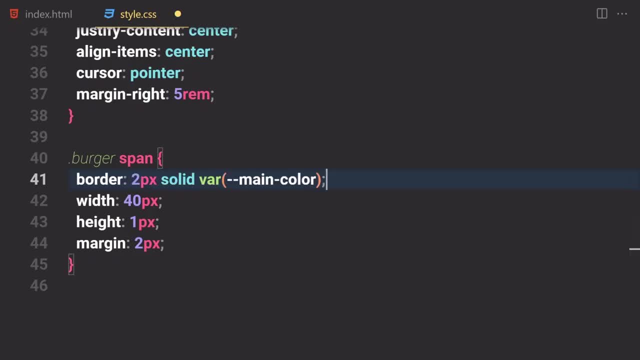 if you comment this one out, nothing will show up. yep, that's looking totally better anyways. so now what else do we have to do? so now let's just start working on our header area. so i'm going to just write first of all: uh, nav ended, or and would be fine. so 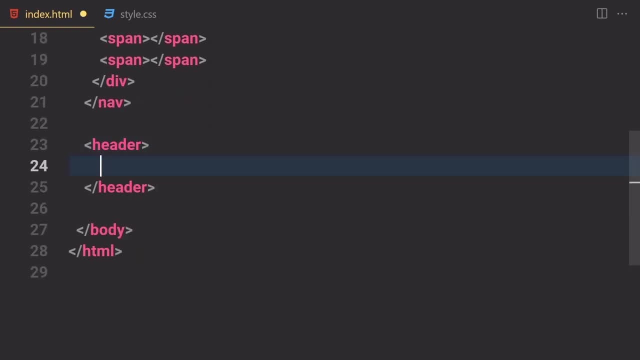 underneath this navigation area. what do we have to do? we are going to be writing a header opening and closing tag. then we have to just write a header content and then, inside this header content, we have to write h1 with a class of main headings, and then new cocktail, and then br. and now let's. 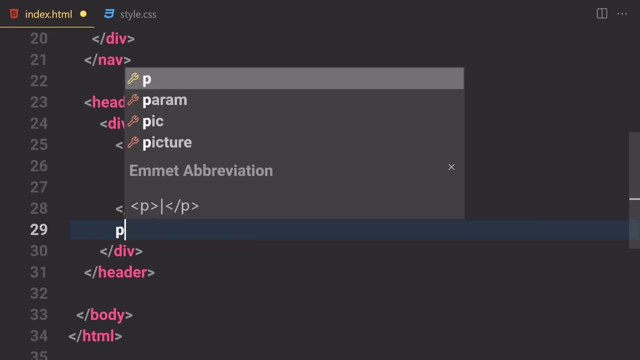 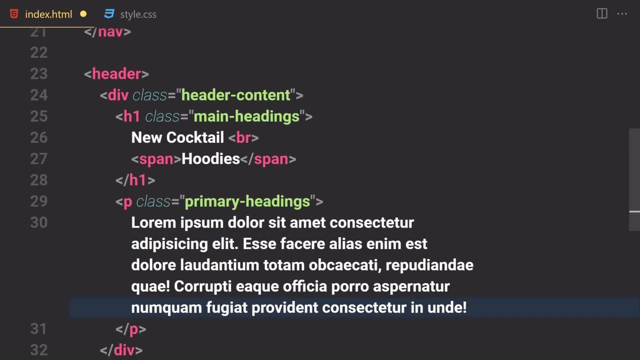 just write a span of hoodies underneath these headings. we are going to be writing a paragraph: uh, primary headings, and now let's just use our lorem ipsum inside there. okay, so underneath this paragraph, what do we have to do? we have to create a container for buttons because we are going to 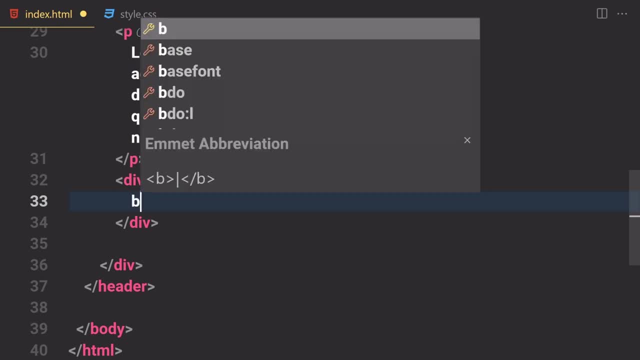 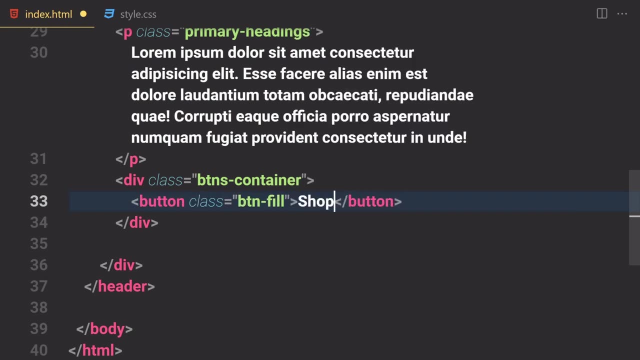 be using a flexbox, so we need to create a container for that. let's just use a button: b? u, double t o n and btn fill. okay, so let's just write sharp. now, this is going to be our first button. let's just create another one which will be 50 off. 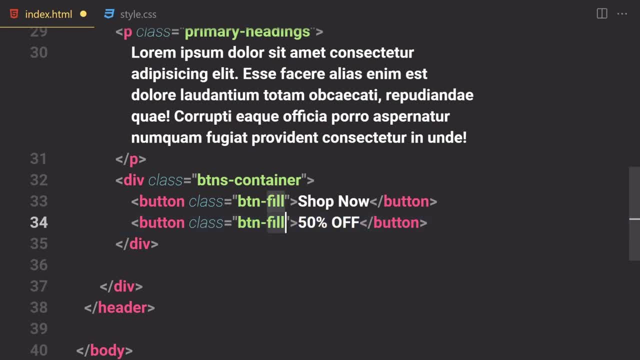 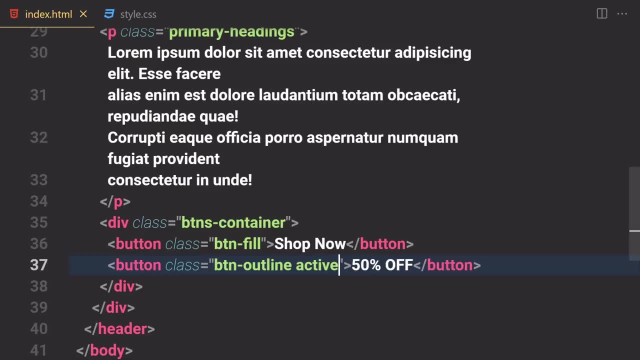 so this is going to be a button outline, so let's just write a button out line and active. this one will be active, the other one will not be active. so this is how everything looks like right now underneath this div. what do we have to do? we have to create another container for our image. 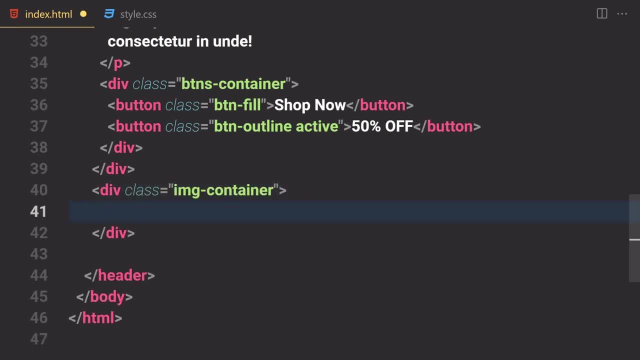 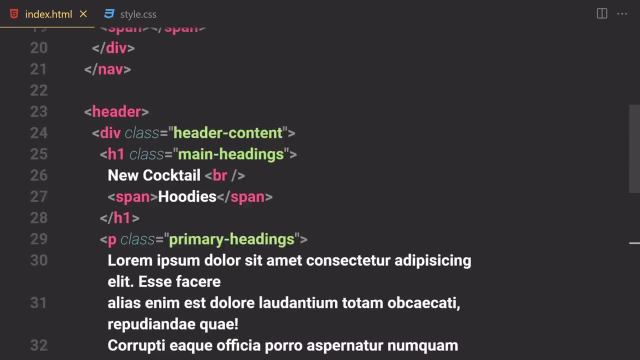 so i'm going to just write image container and we are going to be storing our image inside that container. so we are going to be writing header img for image. okay, so now we are totally done with the html side. now let's just get in to the css side and we are going to be writing our image. 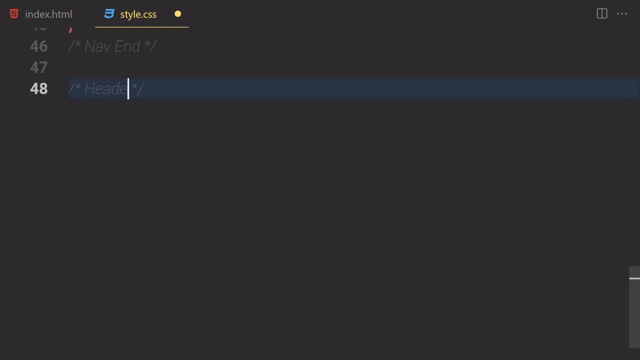 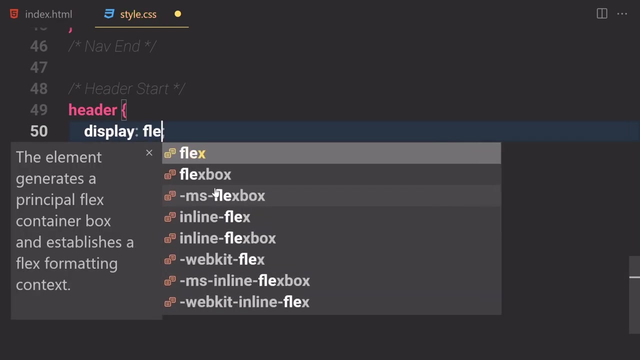 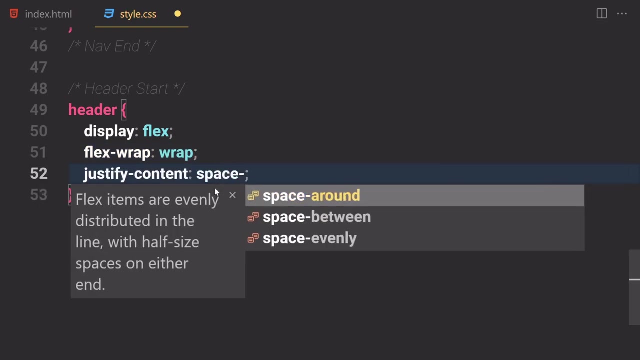 now, let's just style that a bit and let's just write header start: uh, start would be fine. let's select our header. display will be totally flex, uh, flex wrap will be now set to wrap. justify content will be now set to not space. but yeah, i'm going to just set that to space around. align items will be. 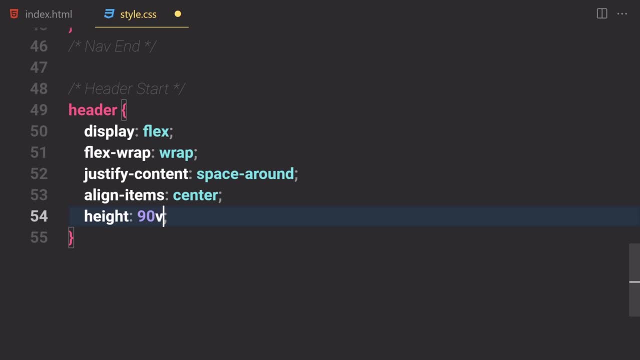 now set to scenery and let's just use a height of 90 vh and margin top will be just two rems, okay. so if you save that- and this is how it looks like now, let's just save that. and now let's just how it looks like right now. okay, so let's just select our main heading real quick. main head. 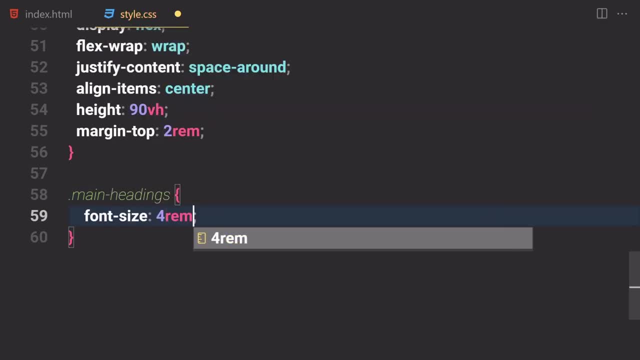 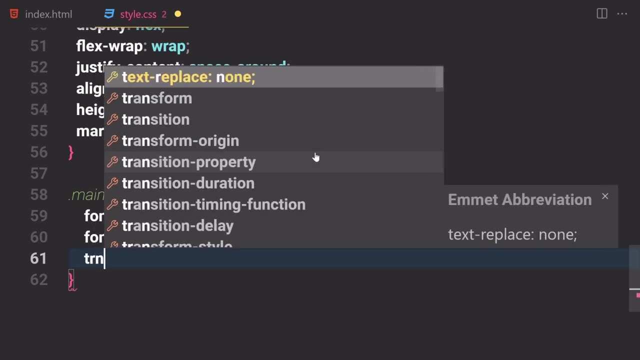 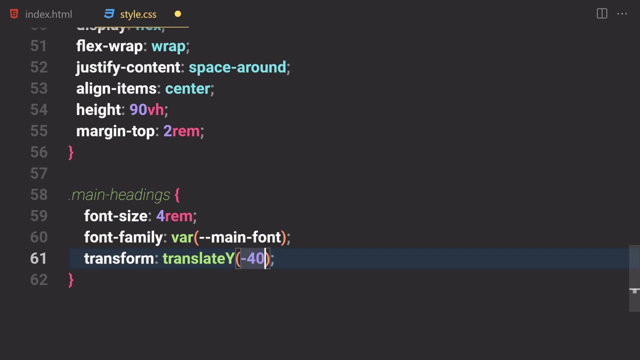 dings and font size i'm going to give like 4m, and for family i'm going to use that same variable which is their main font, and also use a transform and translate it to the y-axis and minus 40, not 500, minus 40 pixel. and now let's just use kind of a oddish. uh, black color. i'm going to select that. 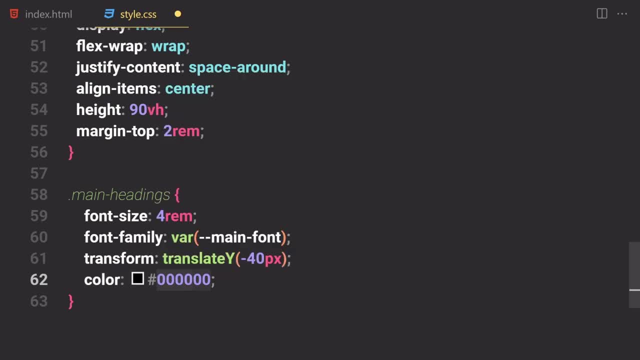 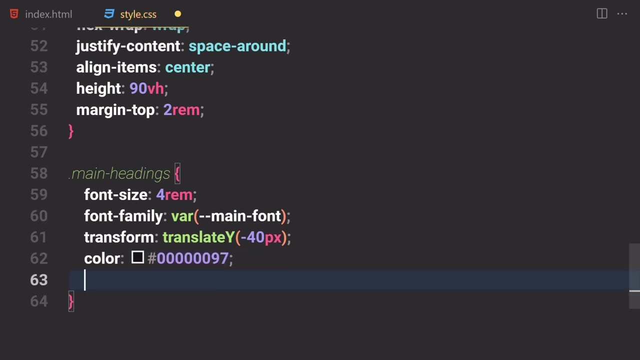 i'm going to change that to hexadecimal values and the last value i'm going to give is like 97, 90, oh my goodness. uh. one, two, three, four, five, six, and then we have a nine, uh, seven. this is going to be the color, and let's just write a line height of five frames. so if you save that- and this is how it looks like- 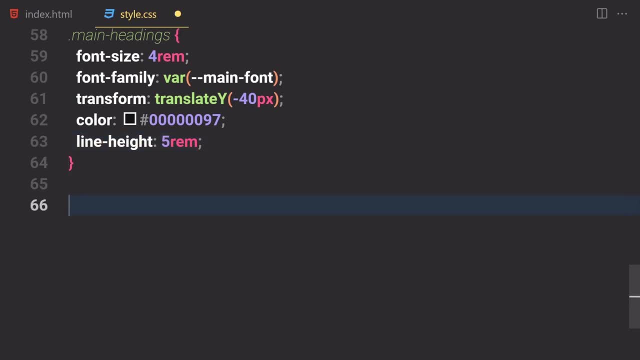 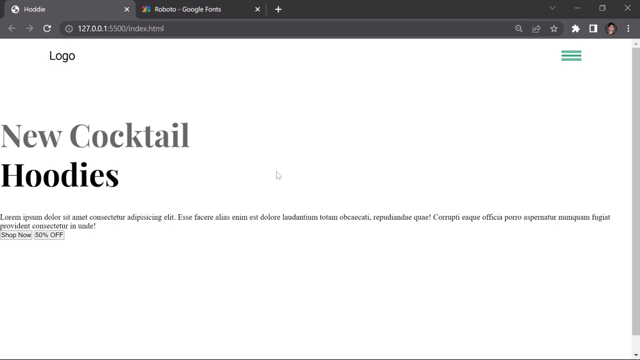 right now. okay, so we just increase the size and stuff. let's just work on our main headings of span, which we provide right here. where is that? this pen which will just select their hoodies? and let's just change the color of that to be like totally black. so, if you save that, and this is how it looks like anyway. so now, 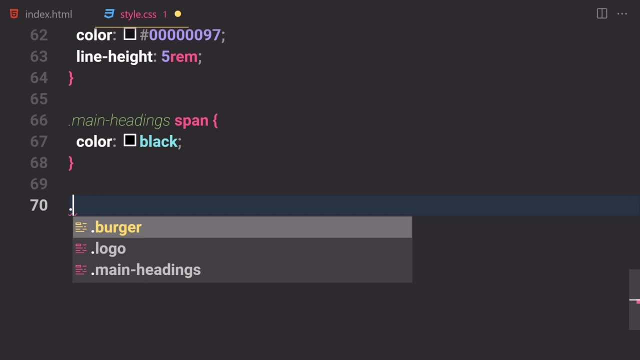 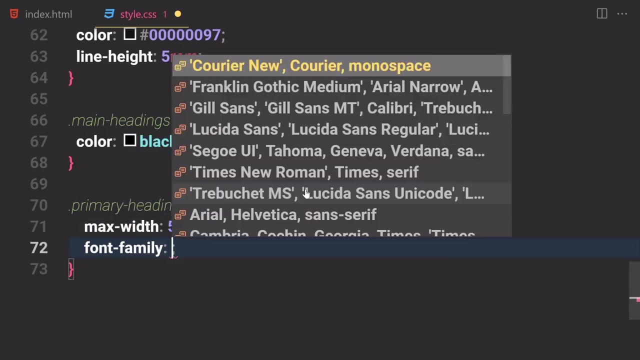 let's just start working on this: primary headings real quick. so we are going to be selecting our primary headings. uh, let's spell it correctly: a p r i m a r y. yep, primary heading, so max width. i'm going to give him like 500 pixels. font family will be totally war and then 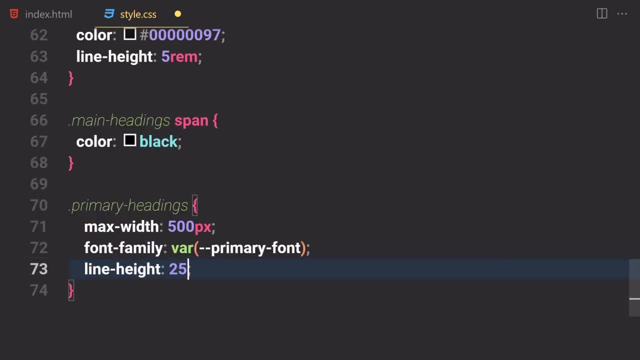 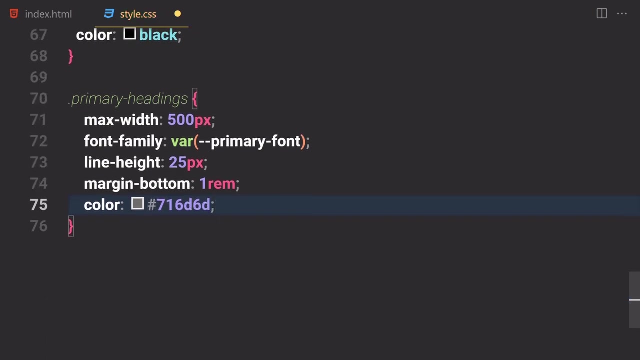 primary font. let's just write a line height for that as well, so 25 pixel would be fine, and margin bottom. i'm going to give him like one rim, and the color which i'm going to be using is 7, 1, 6 d and 6 d one more time. so this is going to be the color, so save it and this is how it. 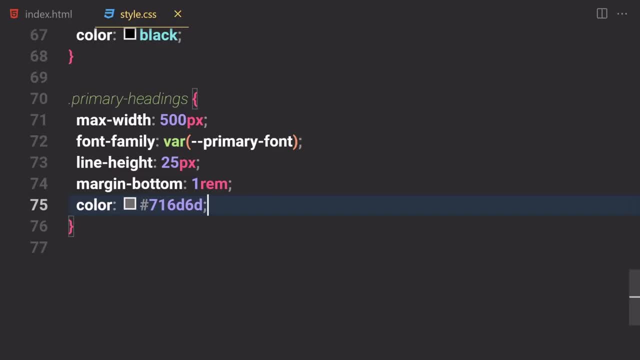 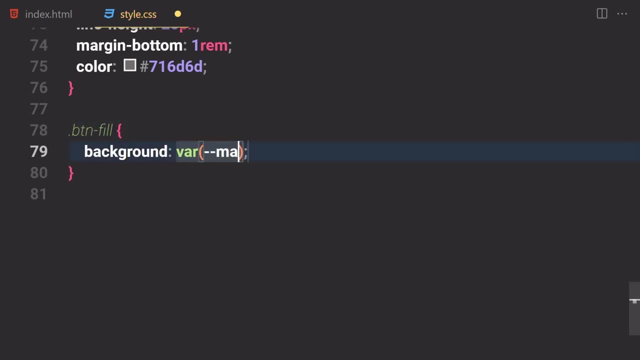 looks like right now. so now let's just start working on these buttons as well. i'm going to select my buttons, so just write a btn of fail and background color, which should be set to totally main color that we just selected there, and color will be totally white. the text: 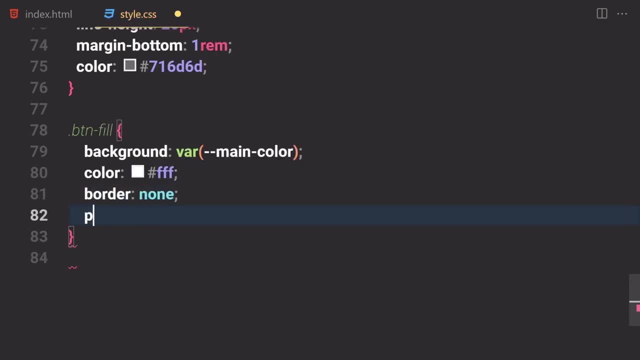 color will be totally white. i'm going to remove their border from him as well. so padding will be for top and bottom 12 pixel, for left and right 20 pixels. so i'm going to also provide a margin right of 10 pixels as well. cursor will be pointer always, and transition i'm going to 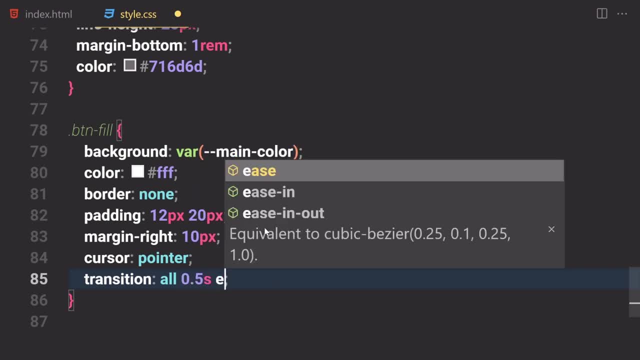 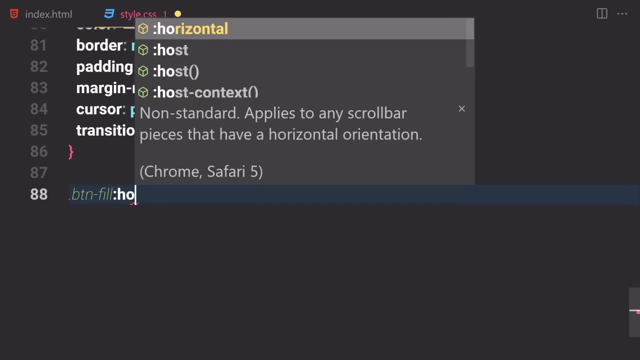 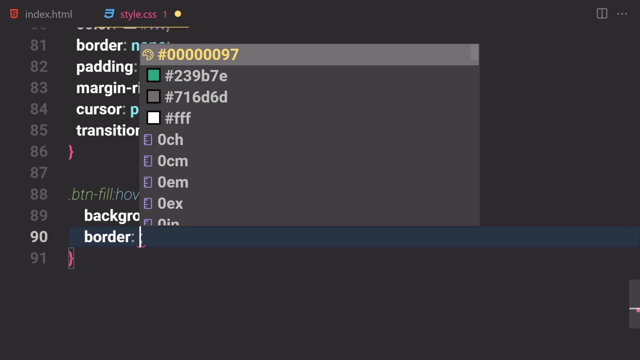 just probably like for everything, 0.5 second ease and out. okay, so let's just use uh hover effect on that. so button fill and once we hover over it. so what do we got to do? we want to change the color to totally white and border. we want to provide a border as well. so one pixel solid and then totally. 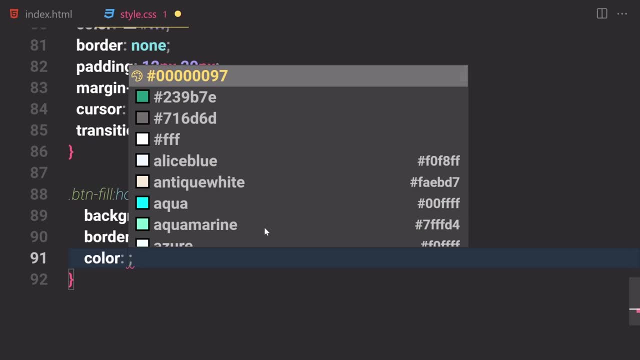 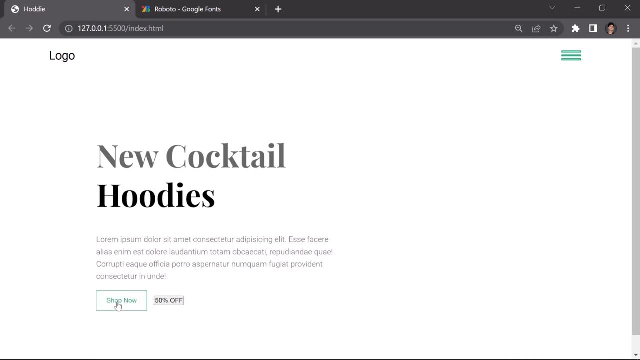 our main color and color. i'm going to change that to like that main color as well. so if you save that- and here is our button, so now if you hover mouse over to it, so here you can see- it will first of all remove their background color. it will now change it to totally white color and we have there. 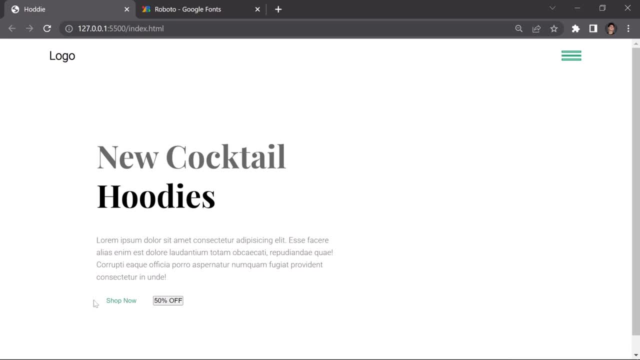 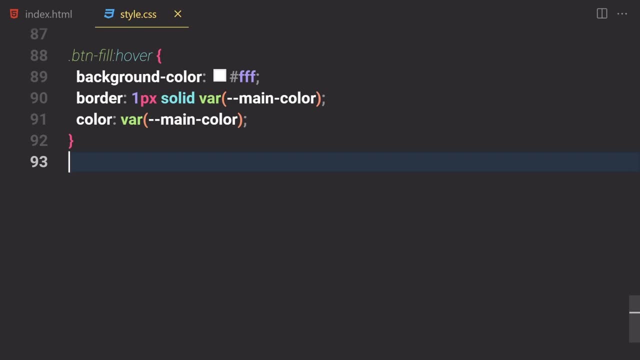 one pixel of border on it and the text color is also changing, that kind of a greenish color which we are using, kind of a main color or primary color, whatever you want to call it. now let's just style the other button, which is the active button, so i'm going to just use btn. 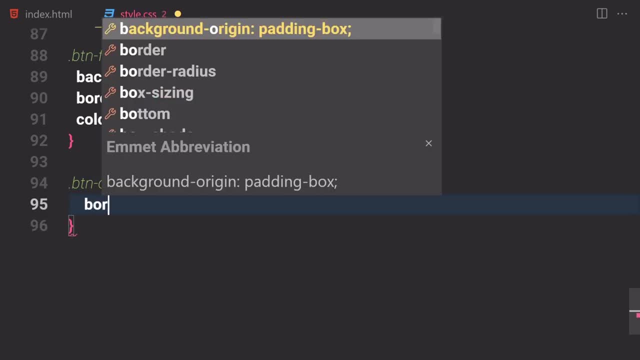 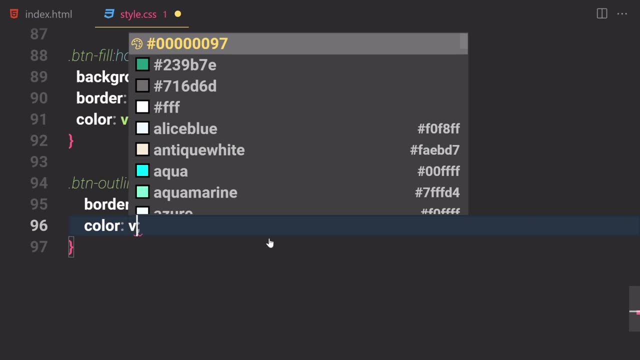 outline and active if that's active. so what do we got to do? we want to write a border of two pixels solid and then use our main color, and let's just also use that main color on this button as well, and background will be now, in this case, totally transparent. 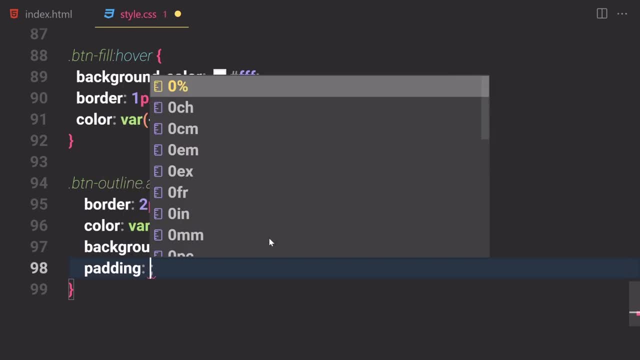 and let's just also use that main color on this button as well. and background will be now, in this case, totally transparent, and let's just also use that main color on this button as well. and background: okay. so padding: i'm going to be providing padding for a top and bottom of 10 pixel for left and right. 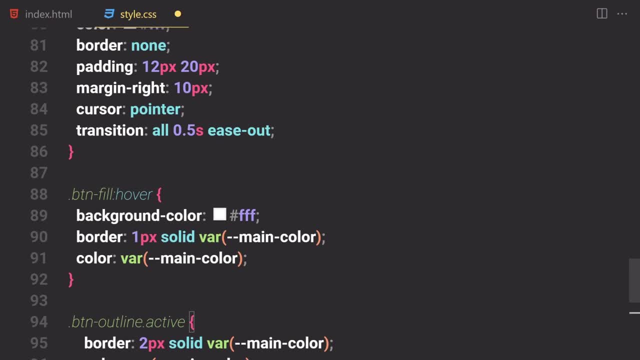 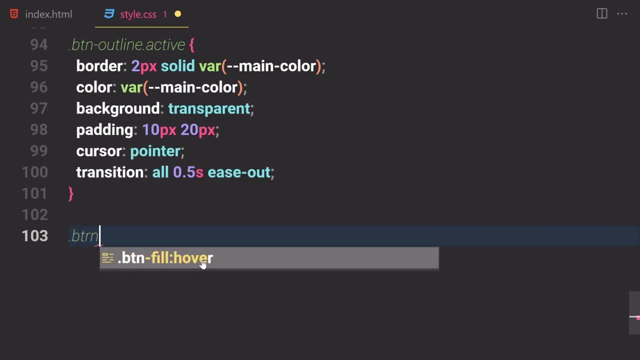 20 pixel cursor will be a pointer, and we can use the same transition, copy it and paste it right here as well. so that's it. so now let's just use our hover effect on that. so btn outline of that active, and once you hover mouse over to it, the background color we want to change is that to. 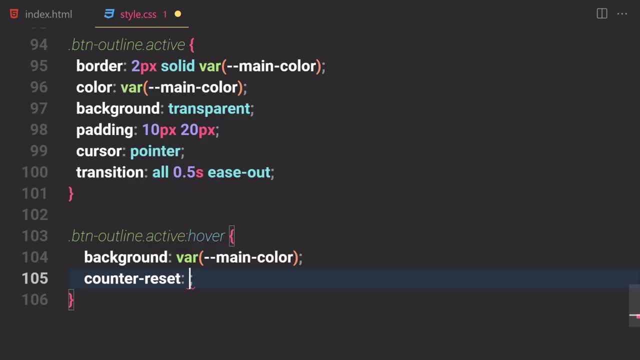 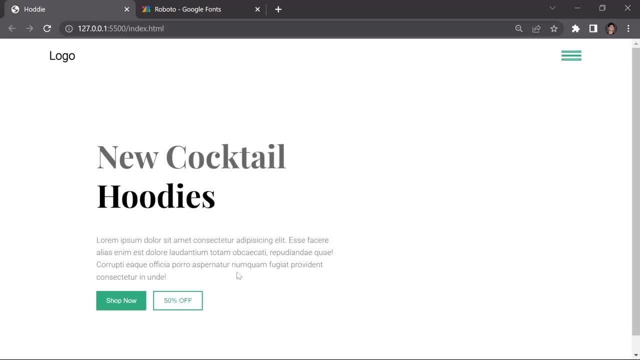 main color which we have as a variable. so we want to change that color of that to totally white. so if you save that- and this is our active kind of a button right here, okay, so i guess that two border, two pixel is a little bit high, but you know what that would do. so we are not. 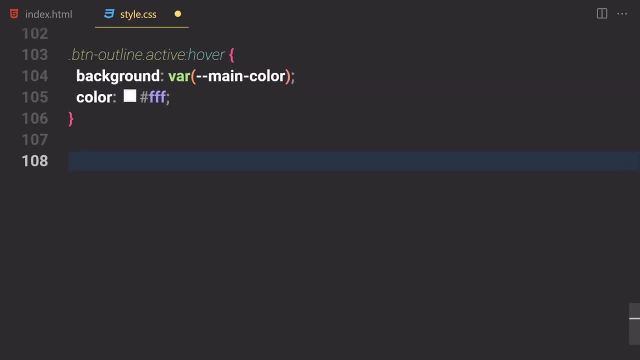 totally done with this section. now. let's just select our image container real quick. so i'm going to just use the like image container. and what do we have to do? i'm going to just write a border radius of 50- uh, 50 percent, and i'm going to also provide a box shadow, not sizing shadow. 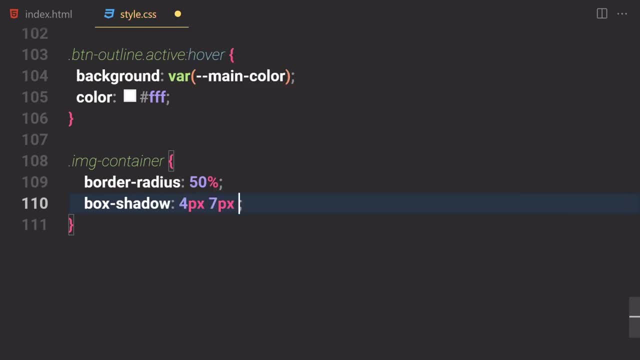 of 50 percent and i'm going to also provide a box shadow, not sizing shadow of 50 percent, and i'm going to just provide a box shadow, not sizing shadow of 50 percent, and i'm going to just write a box shadow of 50 percent and i'm going to just write a box shadow, not sizing shadow of 50 percent, and i'm. 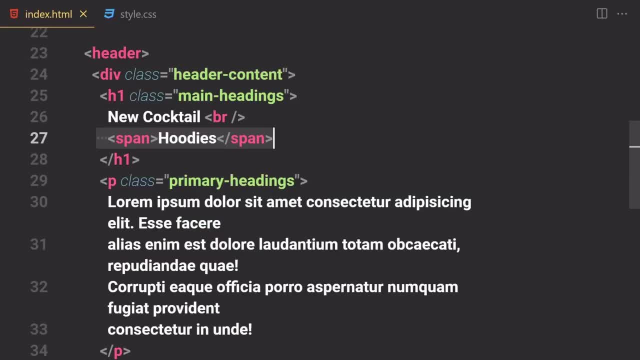 going to just write a box shadow, not sizing shadow of 50 percent, and i'm going to just write a box. now i'm going to just point my finger, so i'm going to just do same thing again. so let's just make sure that everything is, uh, optimized. okay, so we have ourrades node. 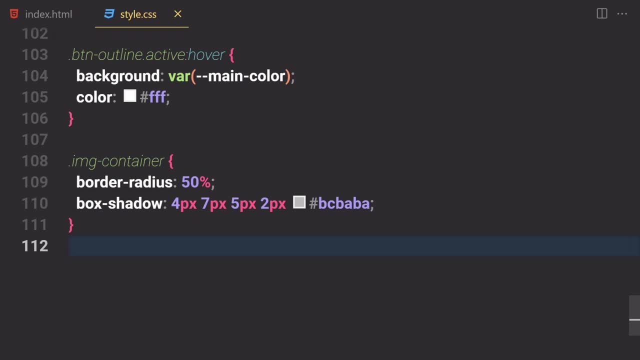 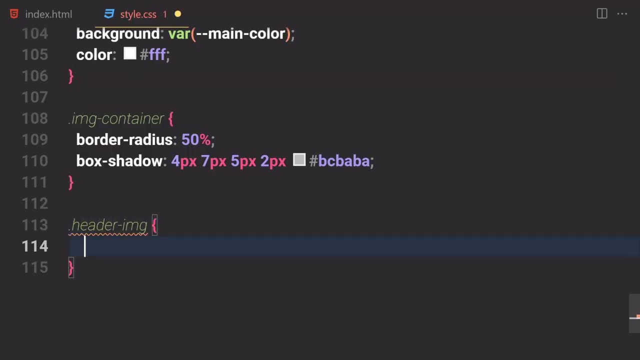 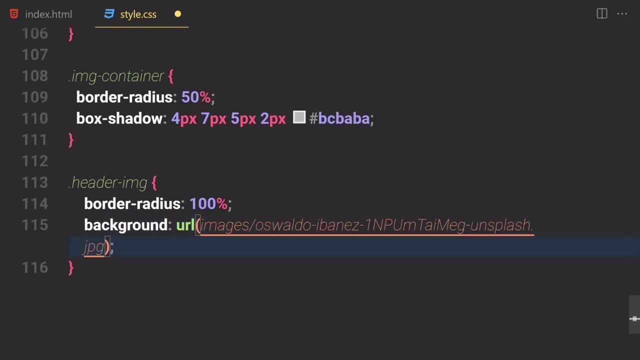 important magnification. collected image content遺損. so in our waitvid form, 확인 unlike, so provide a border radius of 100 on there and i'm going to use a background of url in this case. so i'm going to go to the images section and i'm going to select this image right now and use a. 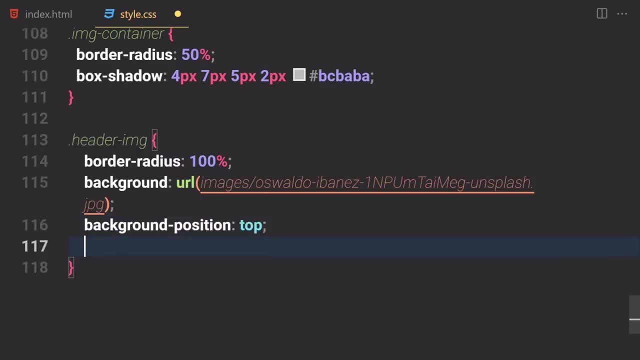 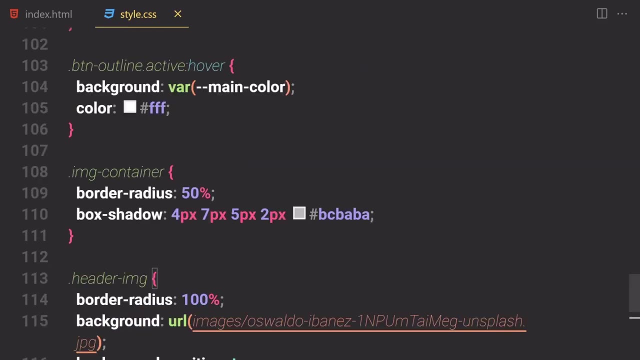 background position to top and also background size will be now set to totally covered, not contains. i'm going to give him a width of like 400 pixel and the height will be also 400 pixels. so if you save that and here you can see, we have this image right here and that box shadow. so if 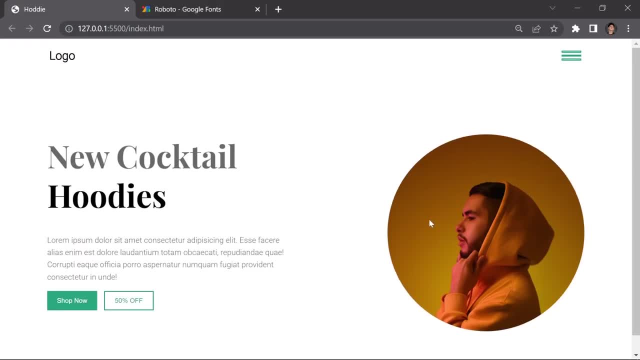 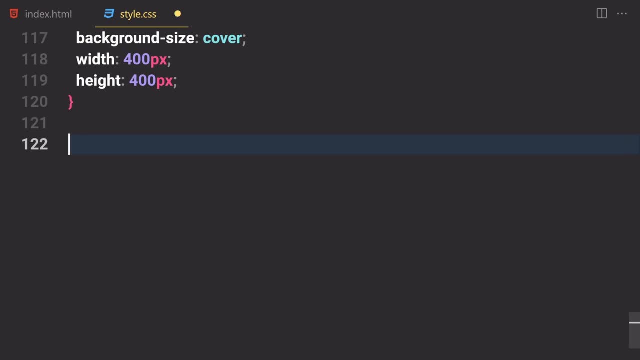 you just comment this box shadow out, save it and this is how the image looks like. if you want to use it, so you can if you like. if you don't like it, so you can just remove it from there anyways. so we are now totally done with our header sections, for header end in this case. so now, 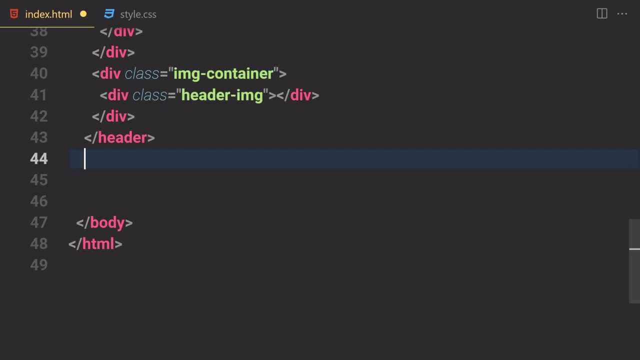 let's just start working on our section one, which is outside from that header. so what do we have to do? first of all, let's just write a comment for ourselves like header and uh yeah, header, and what we find. and now let's just write: or section one start, and here we are going to be creating a section with the class of section. 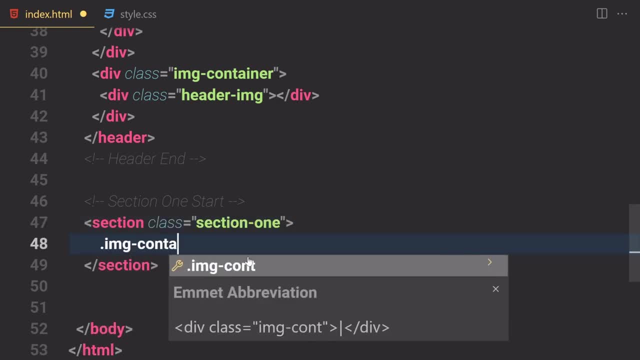 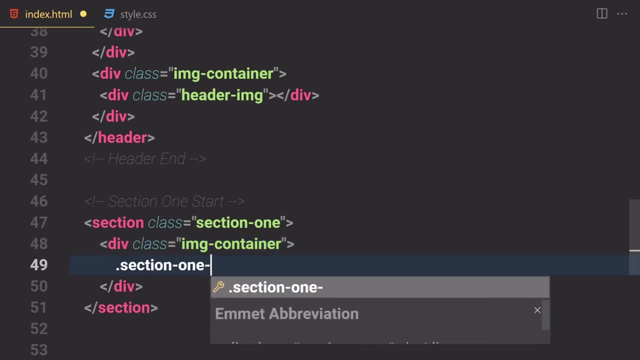 one. okay, so inside there let's just write img and container, like an image container, and inside that image container we are going to be creating a new section one and then img, and now let's just give him another class of header: img. so we are going to 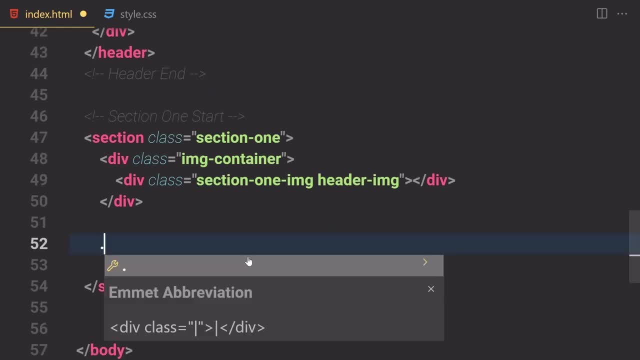 be using their classes and now let's just outside from there. we are going to be creating a new div with the class of section content. so we are going to be using all of our content or we are going to be placing all of our content inside this section. 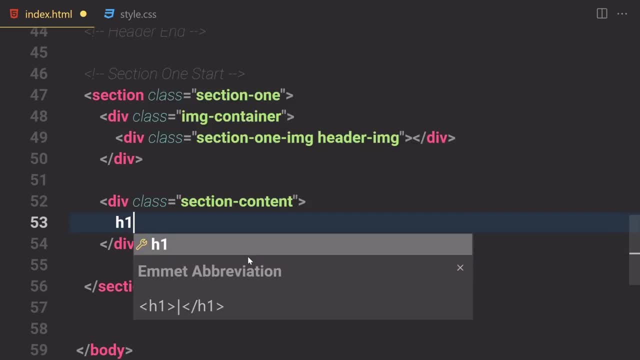 container or section content. why, what am i even saying? so h1, main headings, and let's just write summer and then write a spain with no classes whatsoever. so cell and br. and now what else do you have to do? just write an offer in there, okay, so outside from this h1, right here. 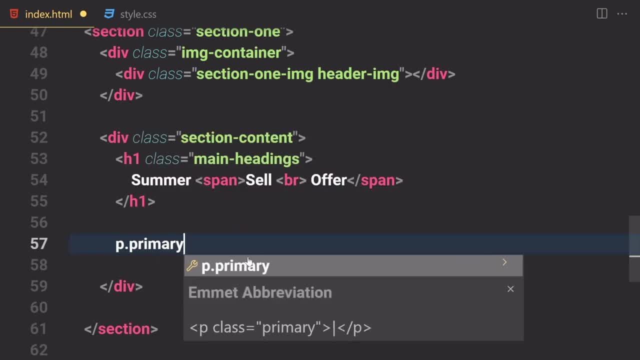 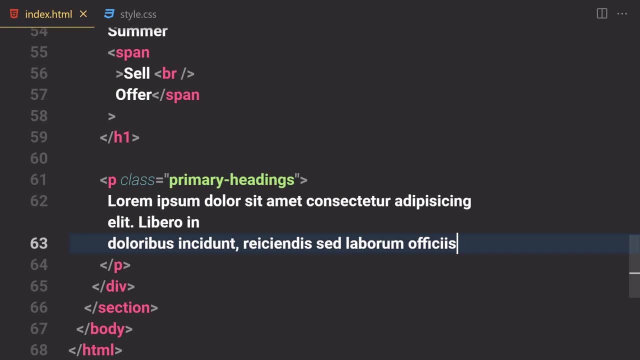 what do we have to do? we have to write a paragraph with a class of primary uh headings, so primary headings, and we are going to be placing our lorem ipsum inside there, but not that much. so i'm going to just write, like maybe two lines of lorem ipsum would be fine. i guess that would be fine. so now, 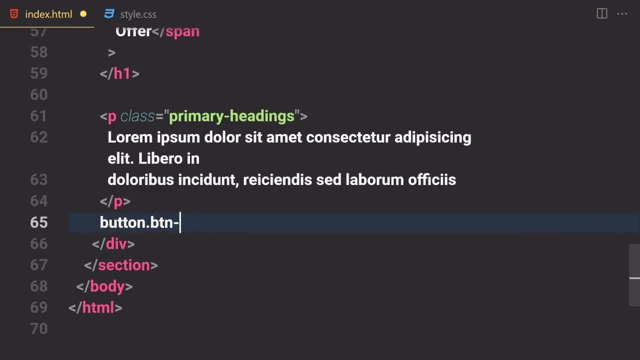 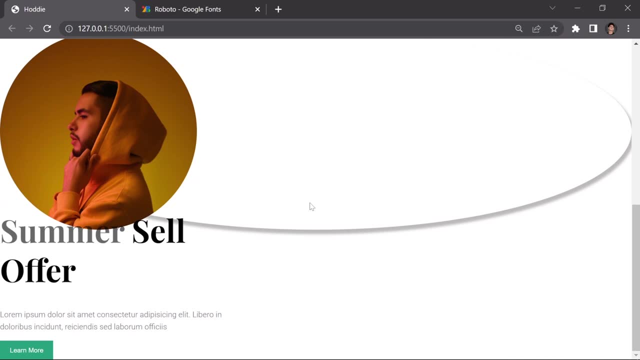 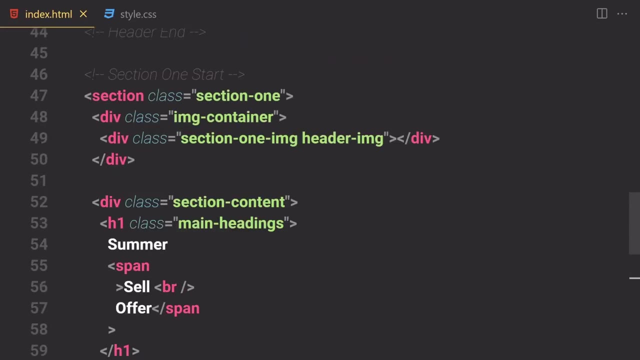 outside from this paragraph, we have to just write a button with a class of btn and fill, and let's just try learn more. so if you sell a file and this- oh my goodness, something that has happened in here- you know what? we will take care of that once we jump into our css. i guess something is wrong. so we have our section one. 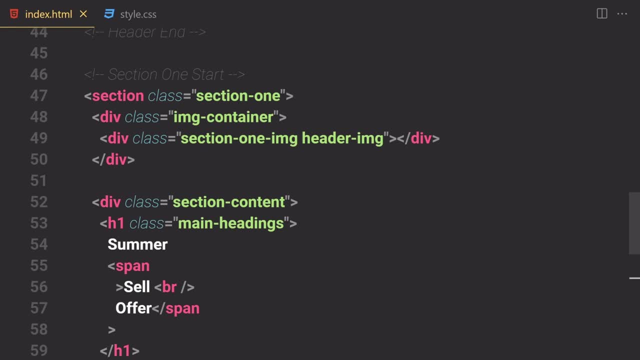 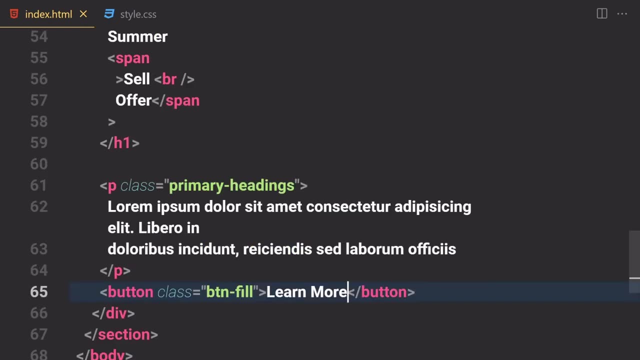 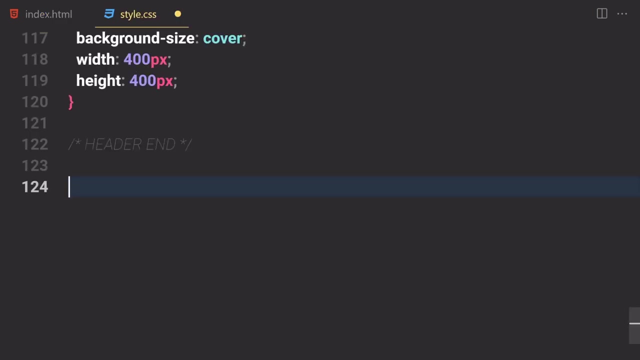 and then we have our image container section- one image- the header image section content. we have our main headings, we have primary headings and then, finally, we have our button fill. let's just get into our css, and now we will take care of that in a second. all right, a section, uh, one start. 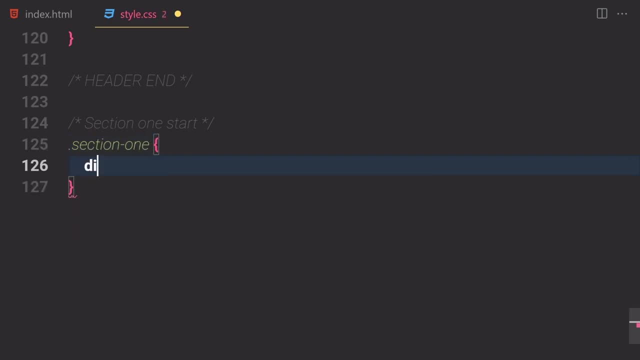 okay, so you're going to be just writing a function one and write a display of flex in here. flex wrap will be now set to wrap uh. justify content will be now set to space around. okay, so online items will be now set to center and margin top. i'm going to give like seven, uh, seven. let me just write: oh my goodness, seven rems. so if you 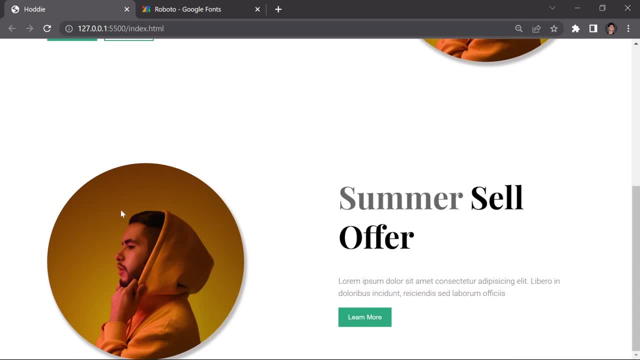 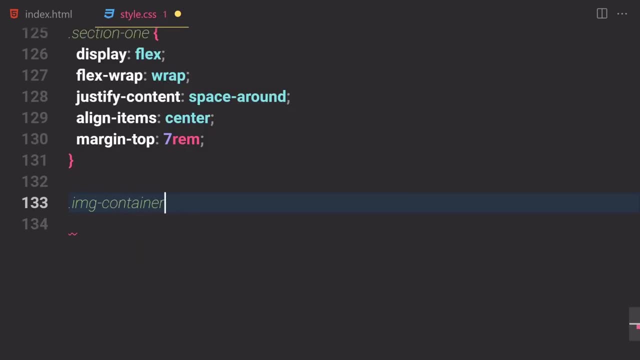 sell a file and this is how it looks like. but we just have to change this image to something else. so you know what i'm going to get into that image container and what should we do here. so we're going to do, we are not going to be selecting that. let's just select for section one, dash img, and change the. 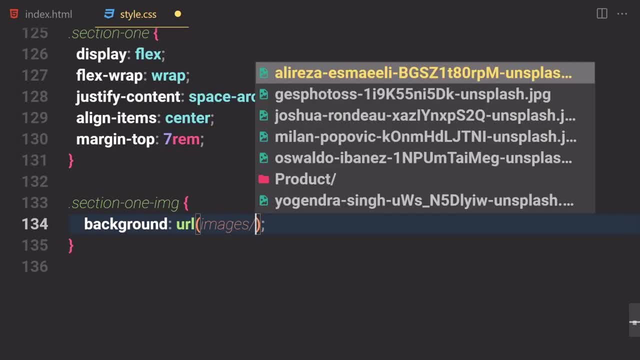 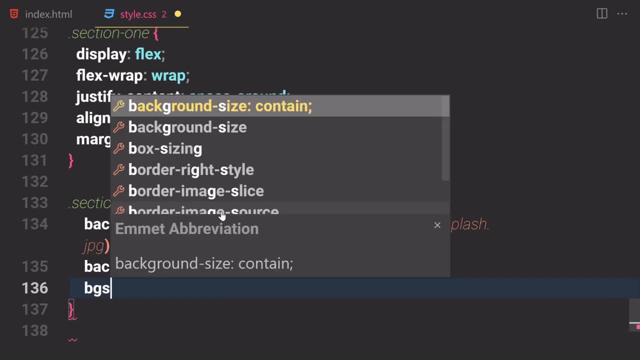 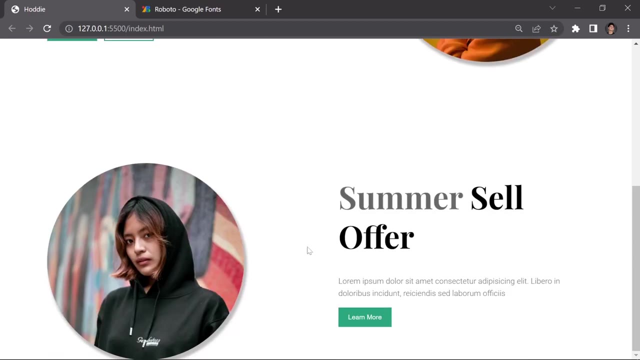 background image to be like something else. so we are going to be selecting for this second kind of image right now and the background position will be now set to top. background size will be now set to totally covered. so if you save a file and now here you can see, we are now getting another image. 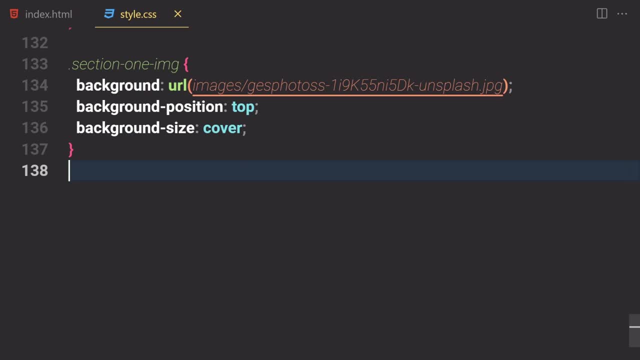 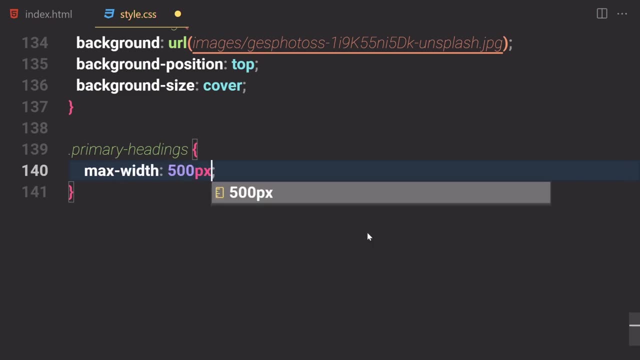 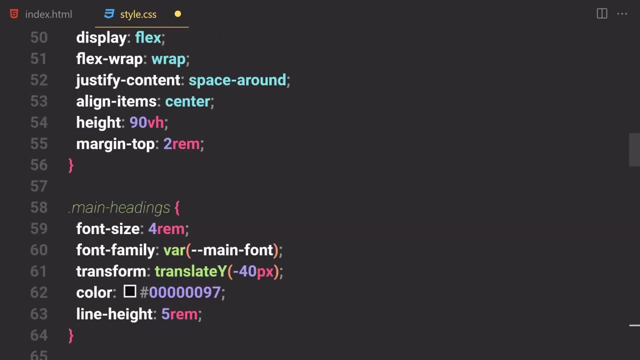 and this is our text and stuff. so now for the headings. i'm going to select my primary headings right now and i'm going to give a max width of like 500 pixels, and i guess i wrote all of this code, uh, right here up above. so let's just search for that primary headings. we. 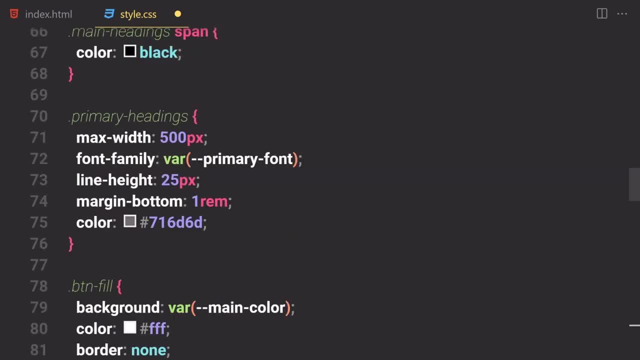 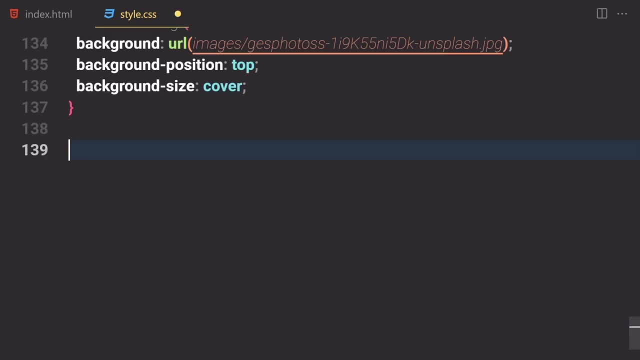 got a main headings and we have primary headings of: uh, okay, so we don't have to write any primary headings one more time. i'm going to remove that and here let me just write like: uh, what, what do i have to write? um, section one, and uh, or end it. would you know what? end is fine anyway. so now let's just get into the product. 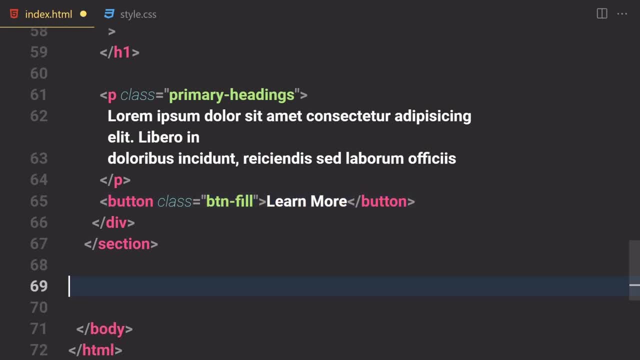 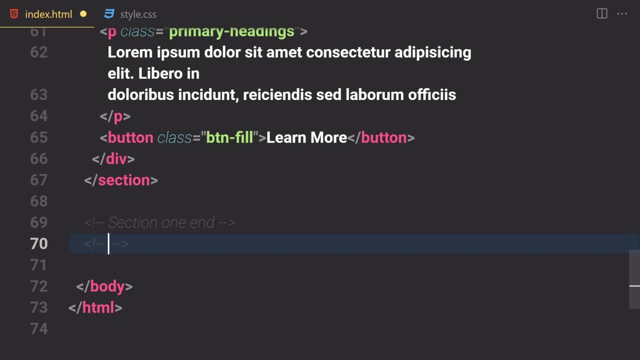 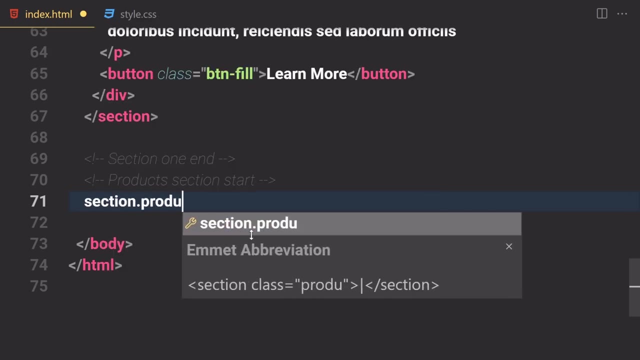 section underneath this section. first of all, let's just write a comment for itself, which will be like section one- end, and let's just create a new comment for itself like products section. start and write a section with the class of products and inside this product section we are going to be writing h1 with the class of products, uh heading. 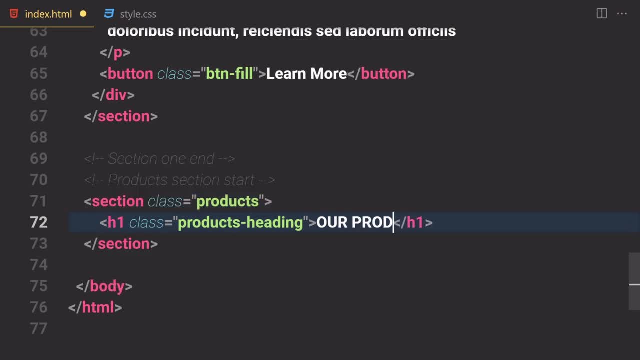 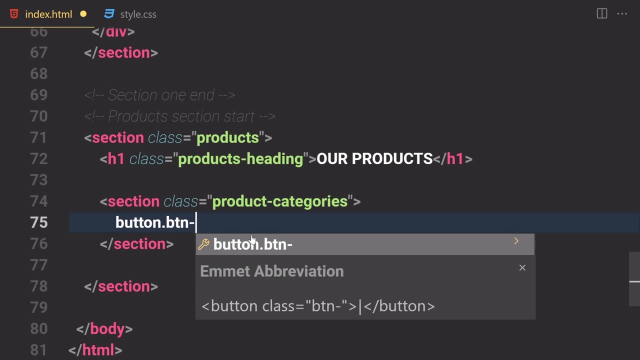 and let's just write order products, pr or d, u, c, t, s or products. so let's inside there we are going to be writing a section with the class of product categories. inside this section, we are going to be creating a button with the class of btn. 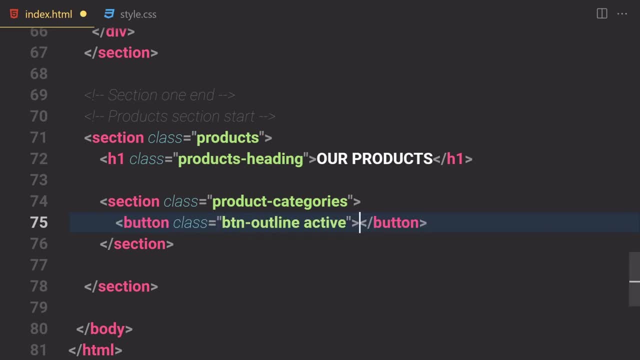 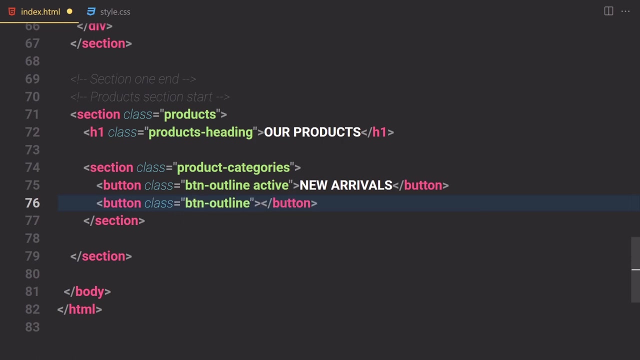 outline and this one will be now active. the first one will be active and new arrival. then let's just create another button. so i'm going to create a button with a class of btn outline of what top rating and let's create another button with a class of btn outline and what best. 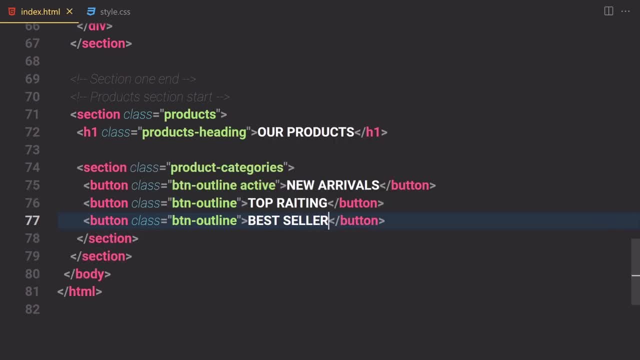 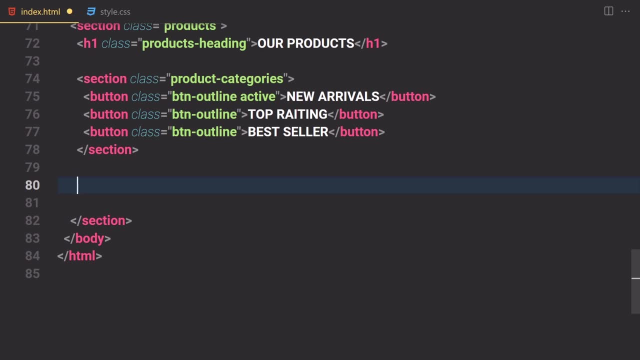 uh, seller, thanks. so we are going to be saving our file for now. but underneath this section, like this button section, what do we have to do? we are going to be writing all of our products item containers, so let's just write like product: uh, items container. so inside the 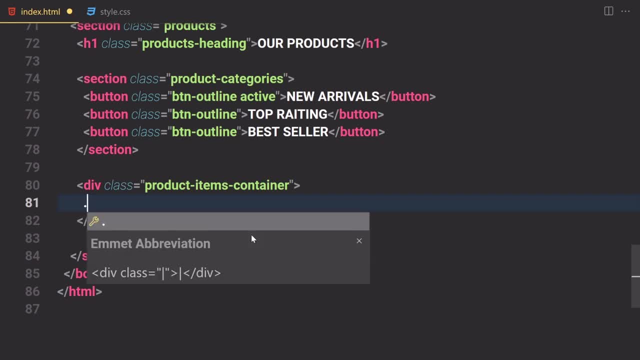 this container, we are going to be rendering, uh, all of our items, so i'm going to just write item inside this item. we are going to be first of all writing item uh layer. inside this item layer, we are going to be placing our image right here. okay, so, uh, let's just remove this r tag from there. 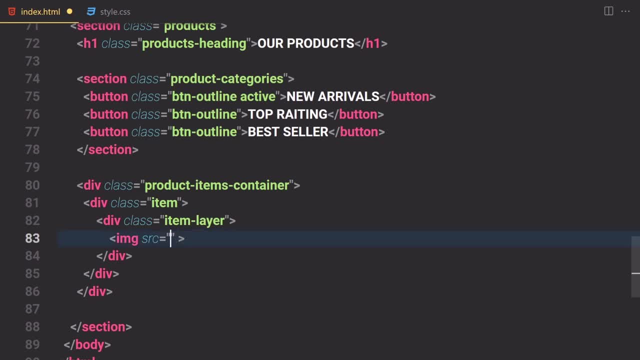 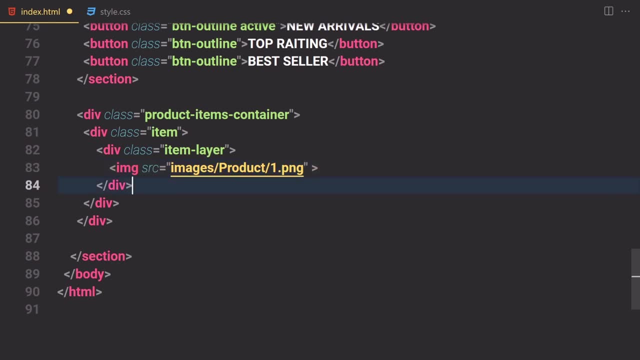 and inside this src, right there, we are going to be using our images and let's just use our product one. okay, so we have our product one. underneath this div we have to write h4 with the class of item name. so write a red hoodie, hoodie and let's just write a paragraph: the class of item price. 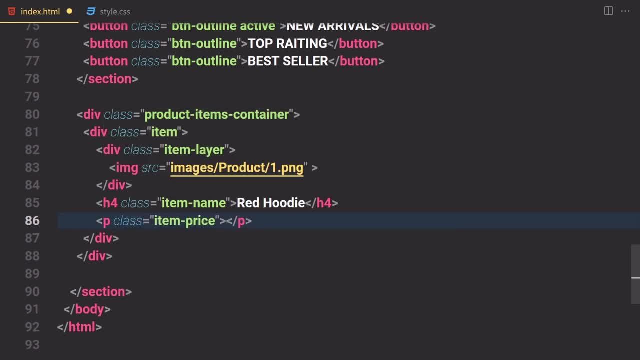 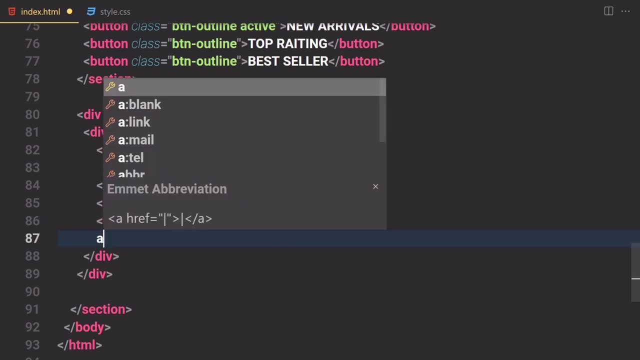 uh, it should be item price and i'm going to just give them like i don't know which kind of price would be fine- 52.99 dollars would be fine- and let's just write an anchor tag, which will go to nowhere, with the class of item name and let's just write a paragraph with the class of item price. 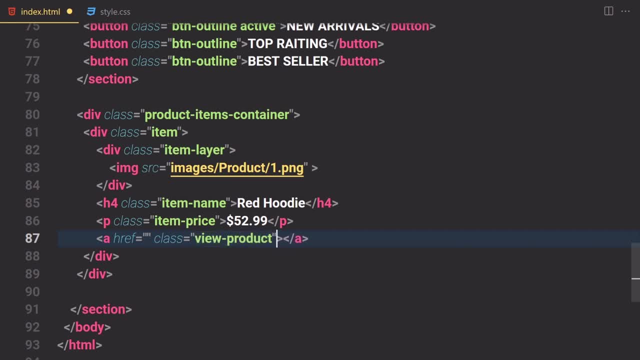 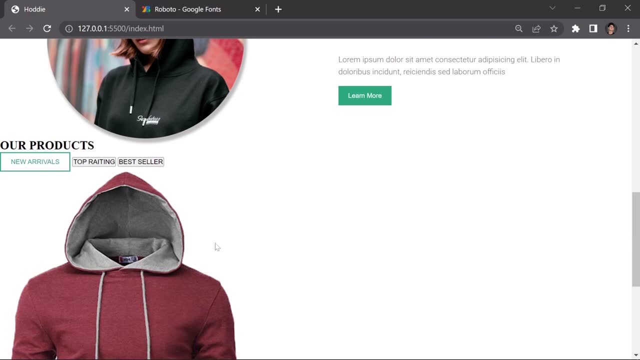 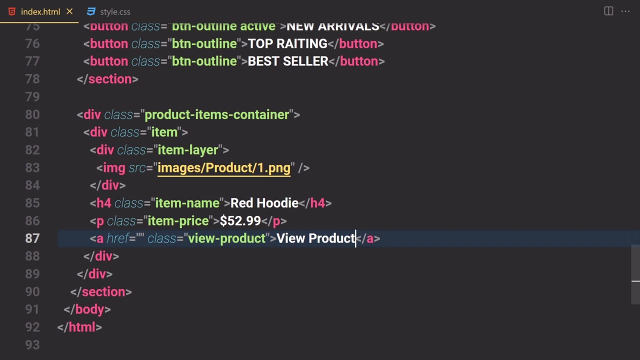 of view products. yeah, our product will be fine view product now, if you sell that. and here you can see we have a red hoodie right here and we have all of these kind of gibberish stuff. but before we take care of that, let's just duplicate our item container, so we have this item container. 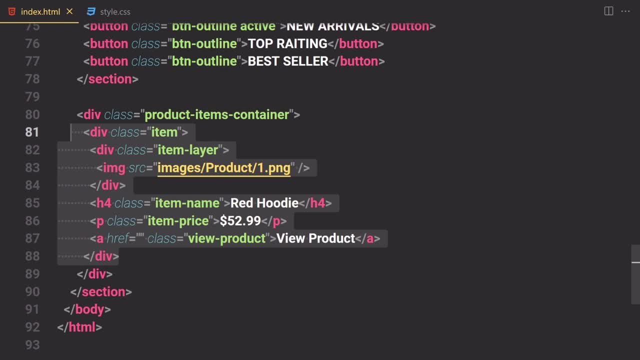 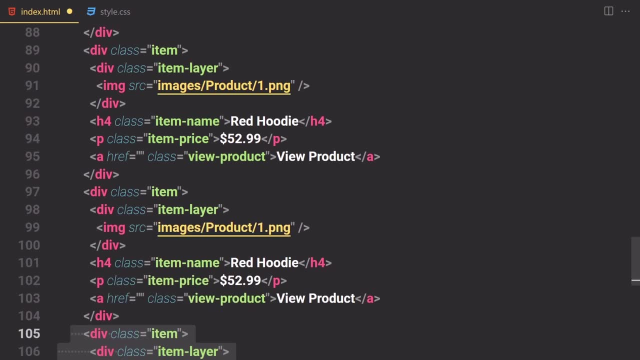 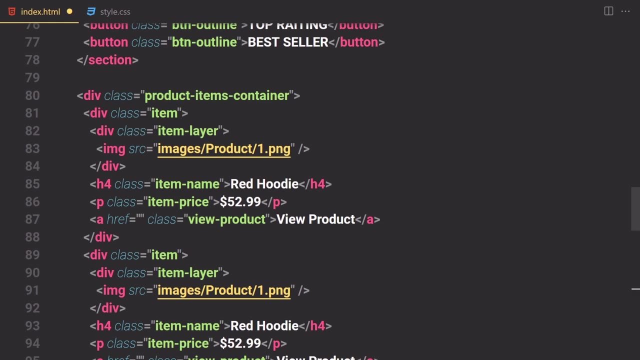 starting from this area. so we have one and let's just create another one. so we have two, three, four, um, and then five, and let's just duplicate one more time like six. all right, so now let's just change the values of them. so we have that red hoodie and that product, so all of the prices and 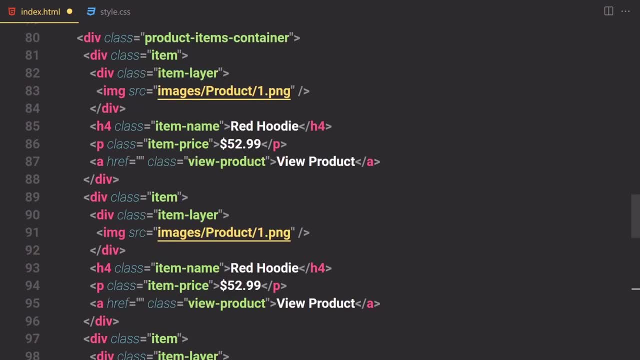 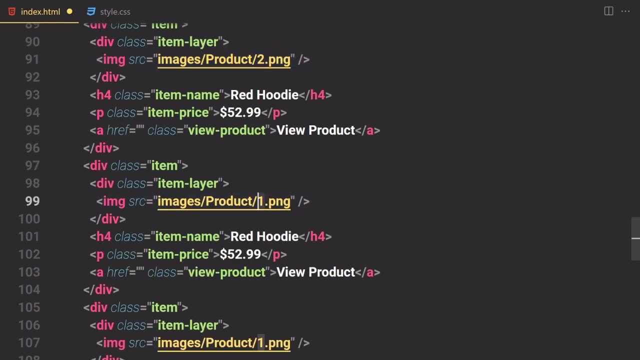 stuff will be the same, but we just have to change the images. we have image one, then we have our image two right here. so what else do we have? we have image three. i'm gonna just replace that with image three, and let's just use that image two right here as well, because we have a lot of images. 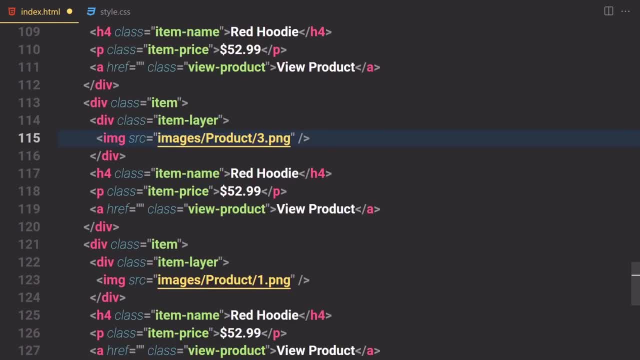 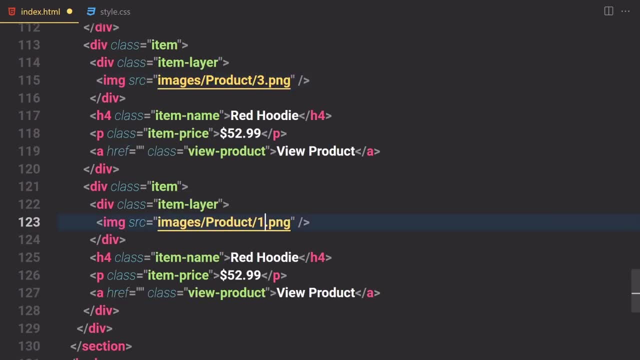 to work with. so i'm a lazy person. that's because we don't have a unique data anyway. so we have three. let's just start working on this one. so this one, this is going to be the first one. so if you sell that we have a red hoodie, black hoodie, greenish or tealish kind of hoodie, then we have 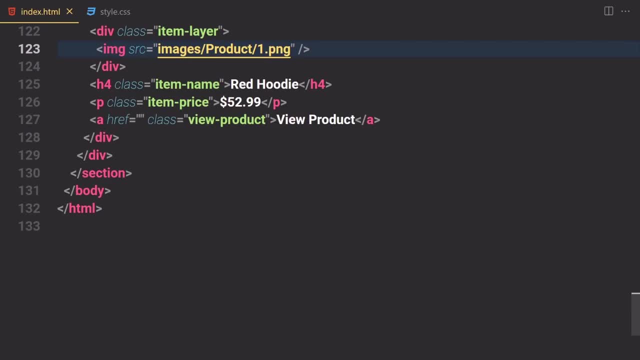 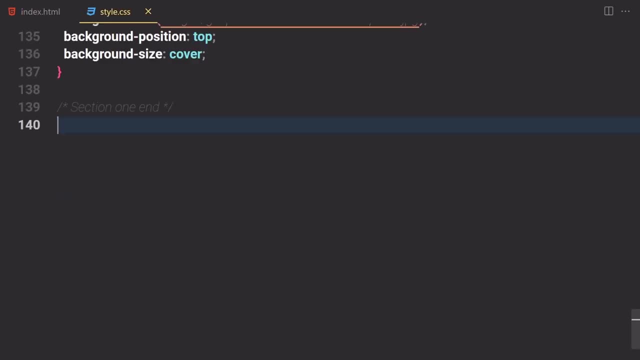 another black and tealish and red one anyway. so now we are totally done with this section. i mean like the html side of this section. so now let's just get into a css and now let's just start working on that. so we are going to be writing a css and we are going to be writing a css, and 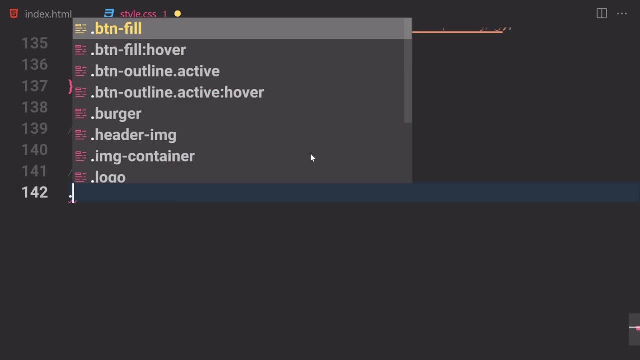 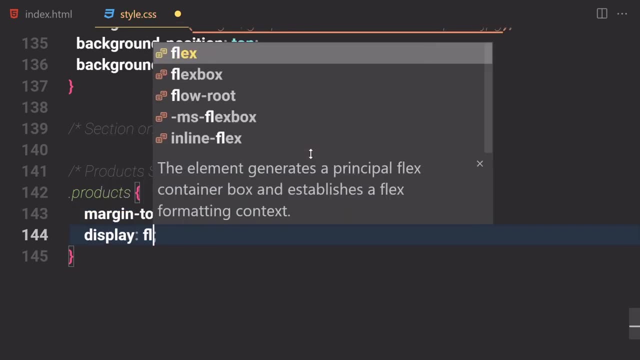 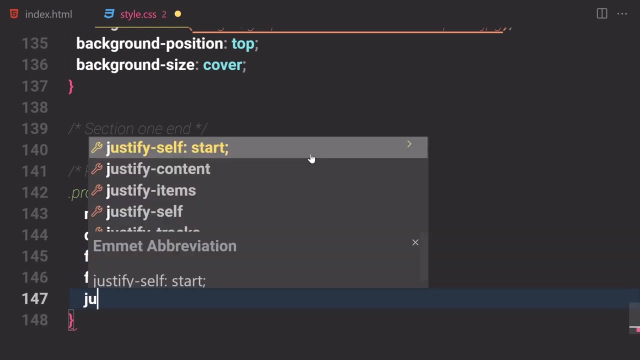 a products. uh, start, and inside there let's just start working on our products. in here i'm going to put a margin top of 10. ram display will be now set to flags. flex wrap will be now set to wrap flex direction. i'm going to set that to column and justify content. i'm going to set that to center. 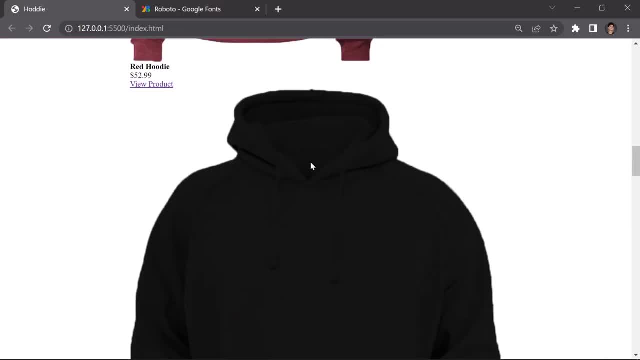 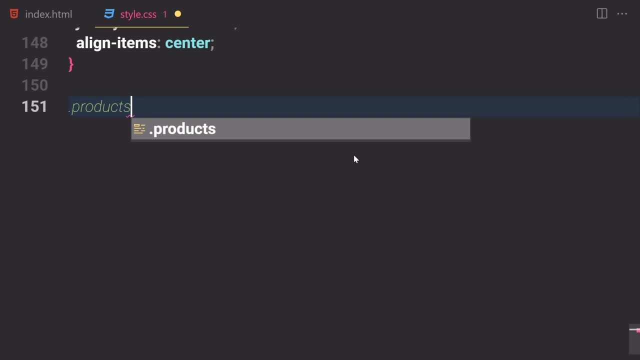 align items will be also set to center. so if you save that, everything is now perfectly at the center, and so is these buttons as well. let's just select our product heading. so we are going to first of all select our products and then we are going to be selecting our products heading, which? 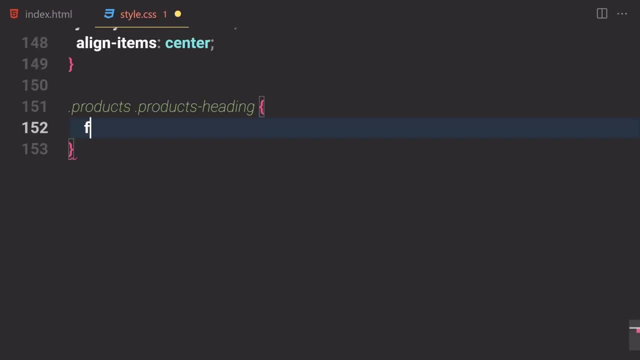 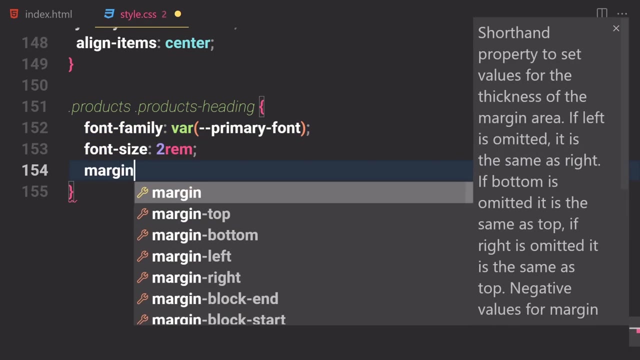 is their product and then product headings. so what do we have to do? we have to change the font family to like a war of primary font. let's just increase the font size to be like 2 ram. margin will be for the bottom. i'm going to give him like 3 ram. so if you save that and this is looking cool. 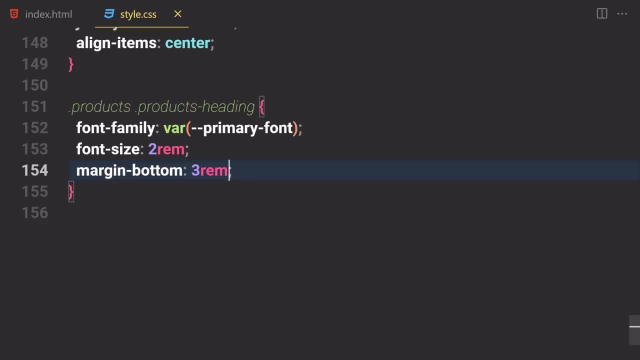 so now let's just take care of the other button, like these two buttons. so let's just select. you know, i'm going to take this select. it's kind of a long one. uh, cut that and paste right here, and instead of heading i'm going to change that to categories. 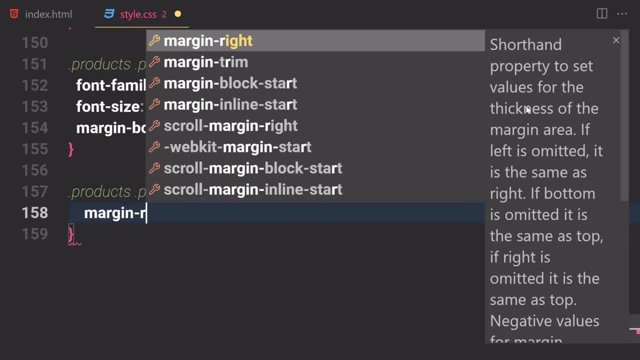 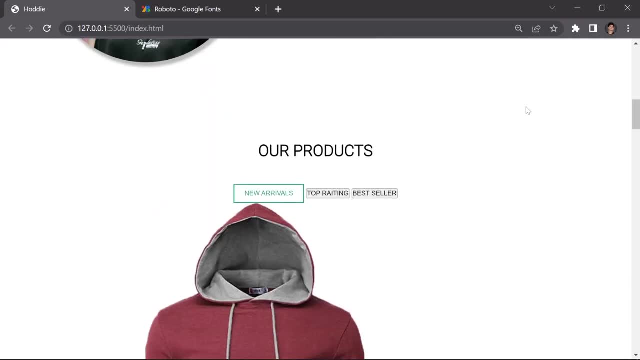 and select our button. i'm going to give a margin right of 20 pixel and margin bottom i'm going to give him like 20, not 20 but 2 ram. so if you save that- and yeah, i guess we messed it up something- c-i-t-e-g-o-r-i-e-s. 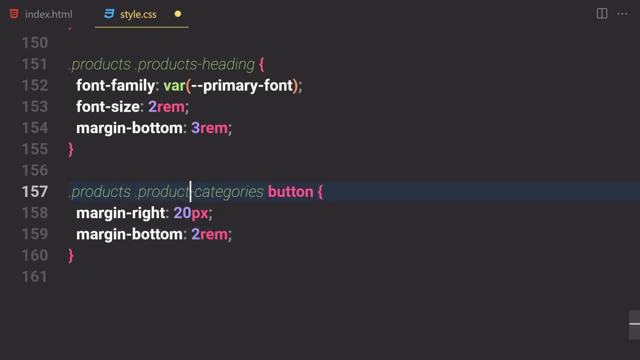 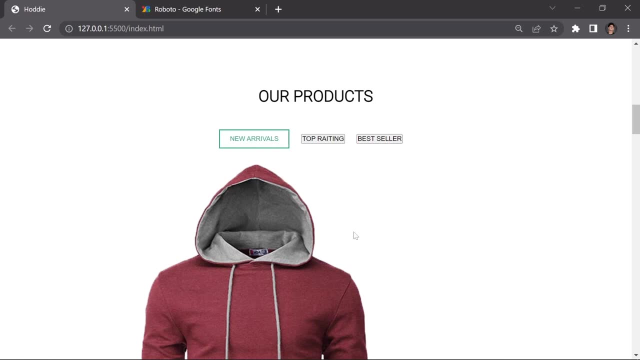 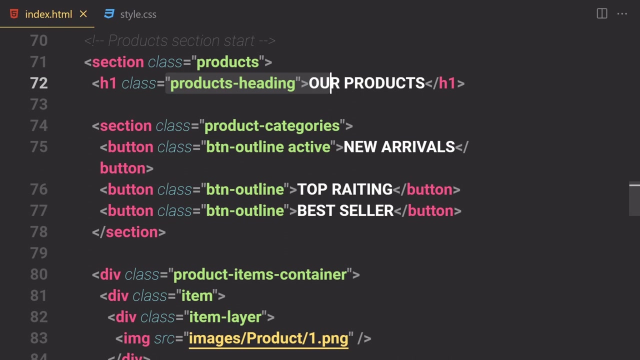 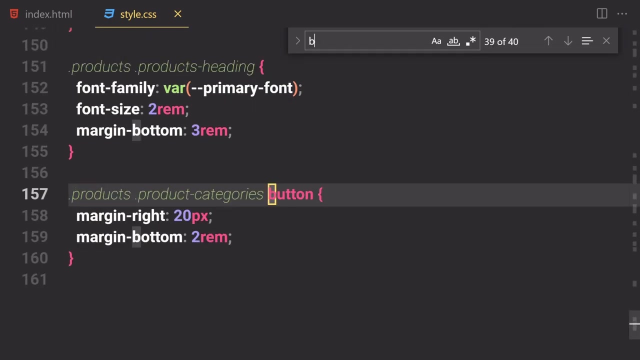 we have products and product categories, not products category. so if you save that, this is something is wrong. so okay, so it's working anyways. um, let's just check our buttons. so we have a btn o u t l i n e outline outline and outlet active. but let's just check btn btn outline. so 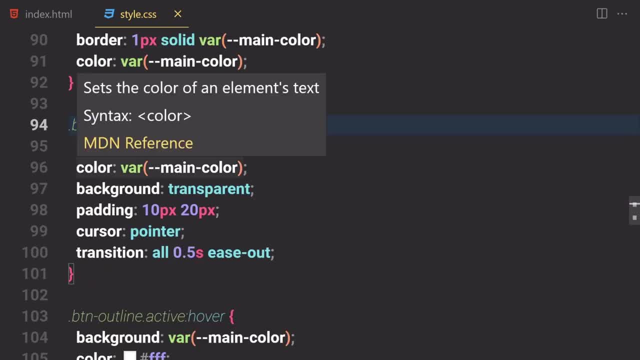 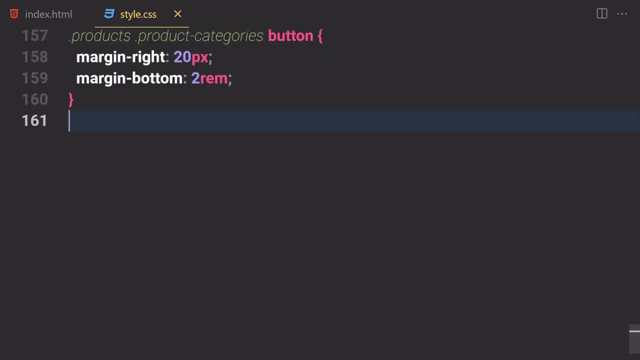 if the product is outlined, then provide active class on there. if not, so what do we have to do? if it's not, you know what. we will take care of their buttons later. now. let's just start working on our products, settings and stuff. so so now let's just select. 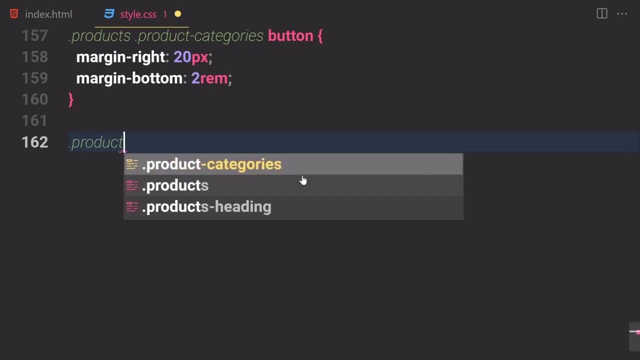 our um products, p r o d u c t s, and let's just select our products, product items and container. which is the product item container which we have right here. i'm going to copy there real quick and i'm going to paste it right here. let's just use our display: flex on it. 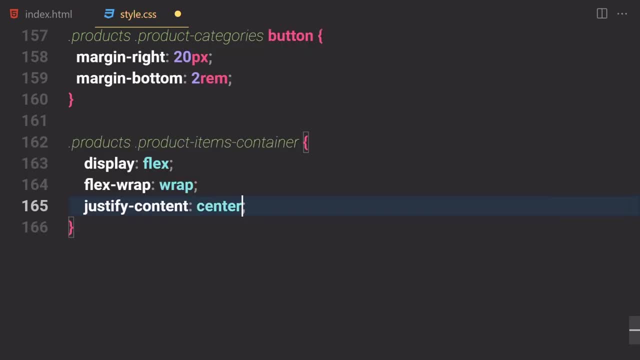 and flex ramp will be now set to ramp. justify content will be set to center. align items will be now set to center margin a little bit, uh, not maximum resolution, but margin will be set to 20 pixel max width. i'm going to give him like a 60 rem, so that's fine. now let's. 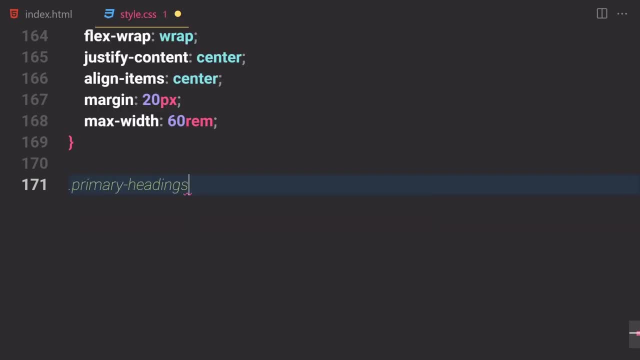 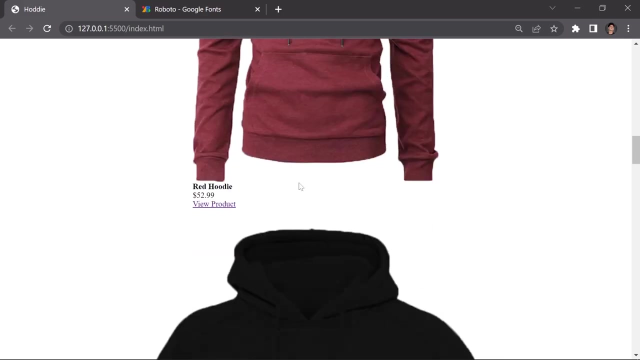 just use a huge uh products. i'm going to use a products and use a product, uh item and container- and now let's just select our item inside there and we are going to be just providing a margin of 20 pixel all around and, yeah, this is looking cool. so now let's just take care of that. 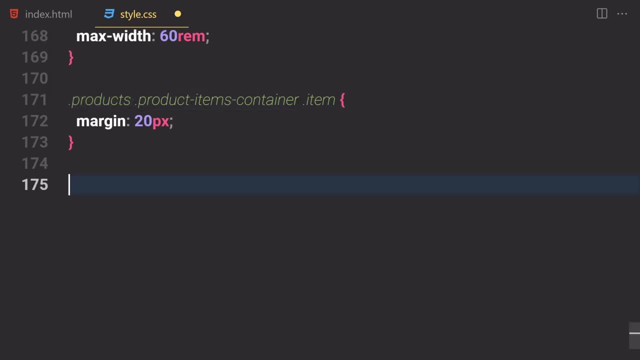 layer real quick. so what do we have to do? i'm going to copy this, i'm going to paste right here and let's just select our item- not item, but item layer to be precise. so, layer and let's just provide a background color of, um, this kind of a different kind of background color: eb, f1, f0 and padding. i'm 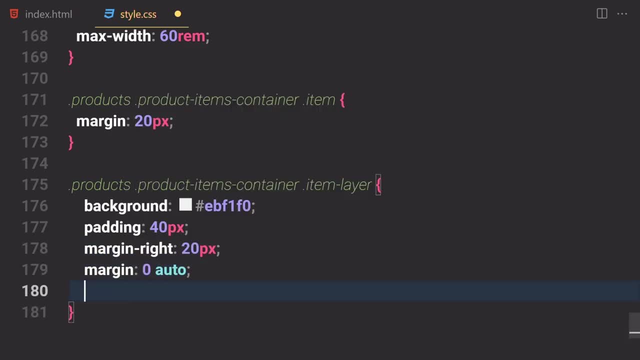 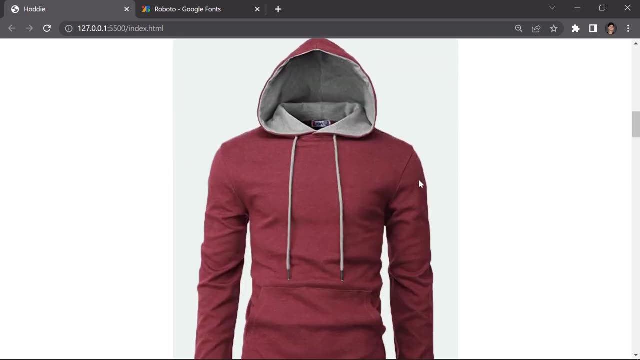 to give him like 20 pixel. margin will be zero auto. so if you want everything to be totally at the center and margin bottom, i'm going to give him like 20 pixels, if you save that. and yeah, we have our products and yeah, this is how our products looks like for now. so this was it for a layer. 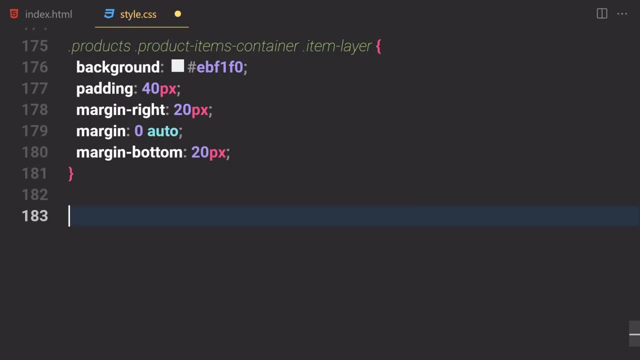 and now let's just decrease the sizes of their images. so i'm going to use a long url- not url, but selector- and we are going to be selecting that item layer in this case, and also you select our image right there. okay, so inside there, we are going to be providing a width of 150 pixel and the 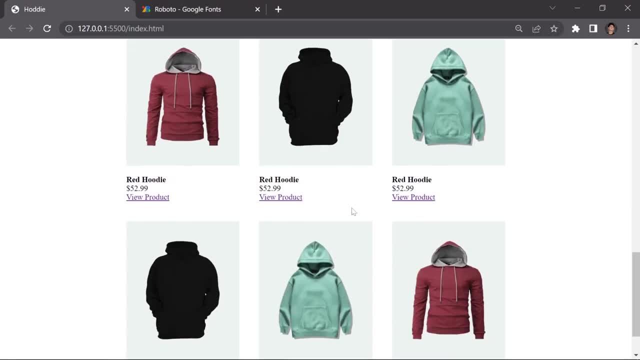 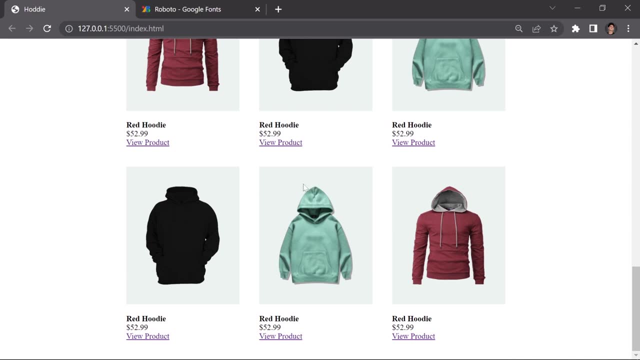 height will be 200 pixels. so if you save that- and this is how currently it looks like right now- okay, so we are totally done with this section, but i guess we have to just style that names and stuff. so now let's just take care of these names. so we are going to be just starting that just a little. 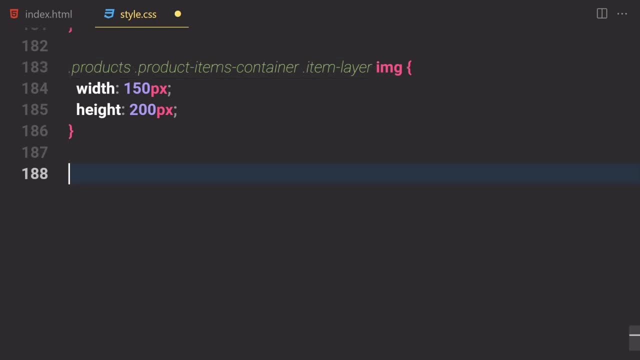 bit. so let's just select everything and use items and not item layer. in this case, we are going to be just selecting item, and now let's just select the item name, okay, so what do we have to do? so i'm going to write a font: family of war, primary font and margin for the bottom. i'm going to give him like 10 pixels. 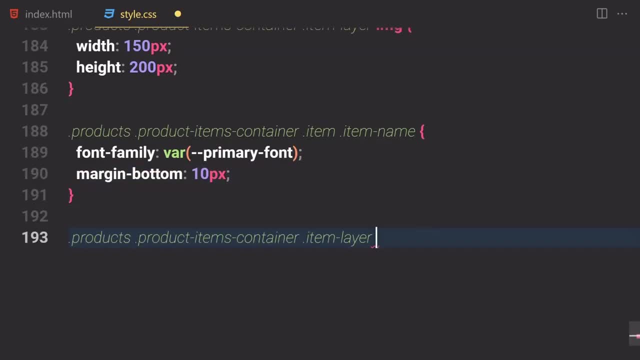 so if you save that, this is how it looks like. and now let's just use that same um selector and instead of item layer we are going to be just writing item price: p-r-i-c- font family. i'm going to change that to war of their not main color. 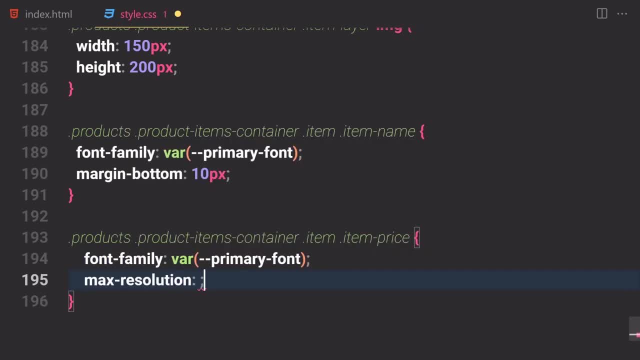 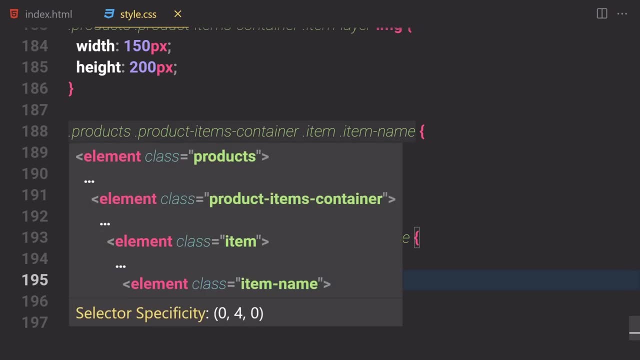 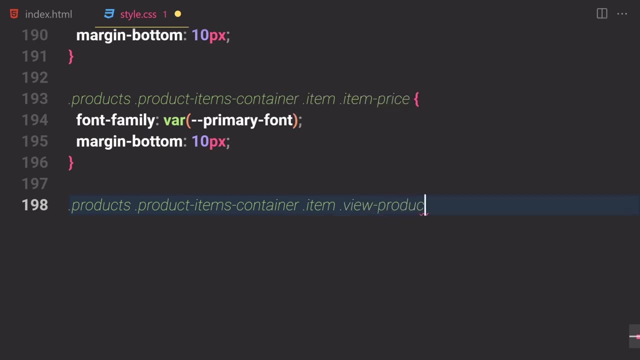 or primary font and the margin bottom. i'm going to give him just a little bit of margin bottom in this area as well, so like 10, pixel 7, and this is how it looks like anyways. so what do we have to do next? we have to select that item and view product. okay, v-i-e-w. yep, the spelling is correct. 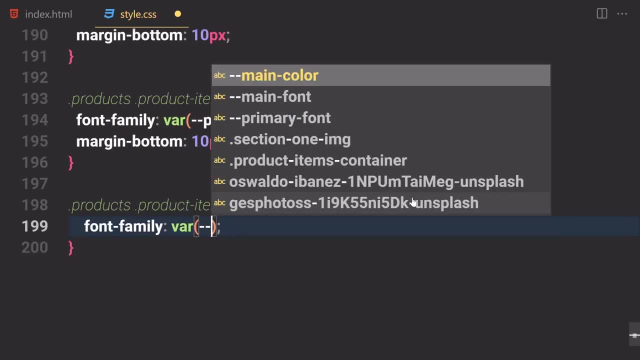 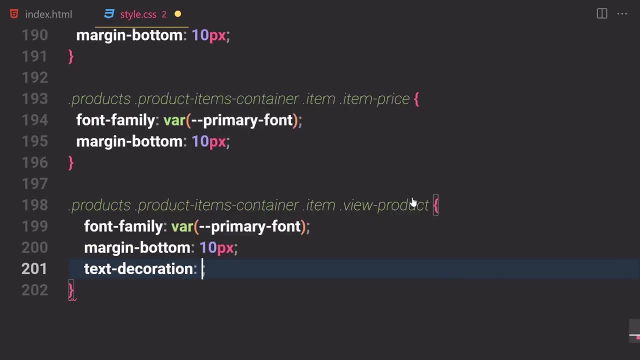 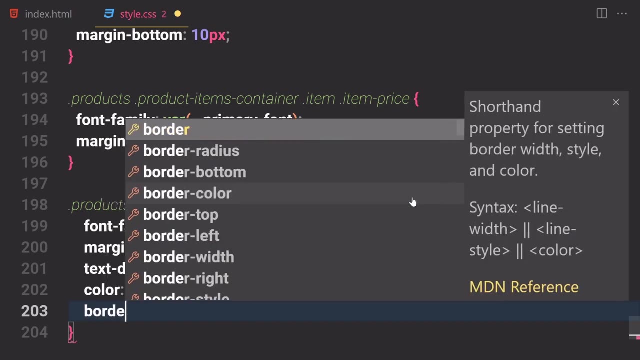 font family will be also using that. um, what is a primary font? and margin bottom? i'm gonna give him like 10 pixel and text decoration- i'm going to remove that. and color: i'm going to use that main color of the variable and border for the bottom, i'm going to provide one pixel solid. 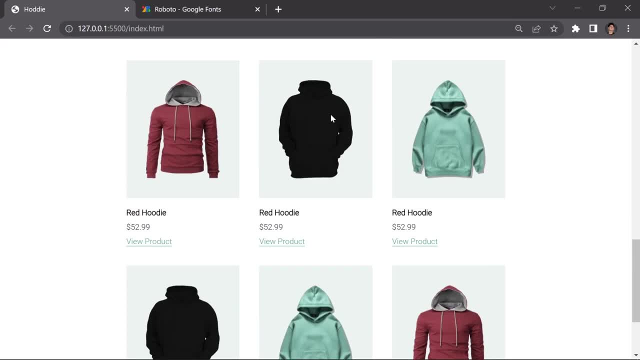 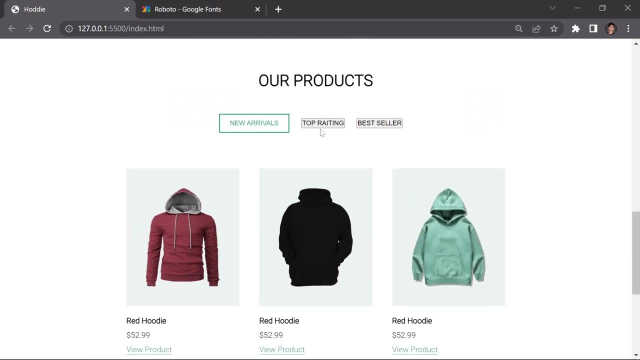 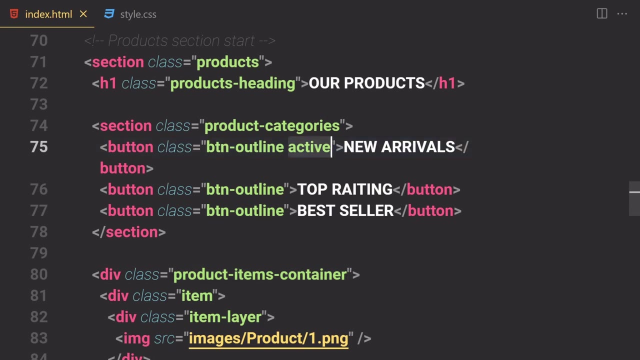 and then war. let's just reuse our main color. okay, so this is now how it looks like right now. okay, so this is looking better, and i'm wondering how can we change this one to something else, maybe. so let me just take care of these buttons real quick, so i'm going to cut this. 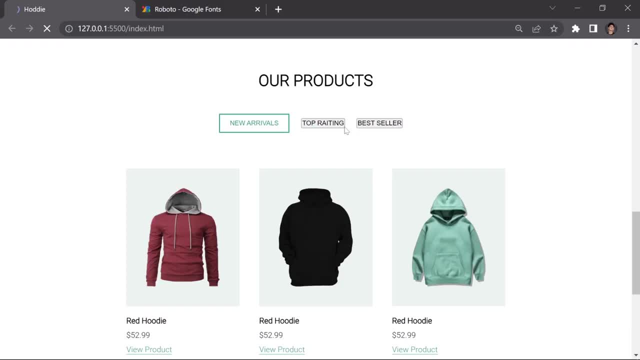 or you know, i'm going to paste this active on these as well, like so. and yeah, that's looking better. so you can just click on that if you want to, or you can provide different kind of styling for that. so you can also provide different kind of styling for that if you want to. anyway, so we 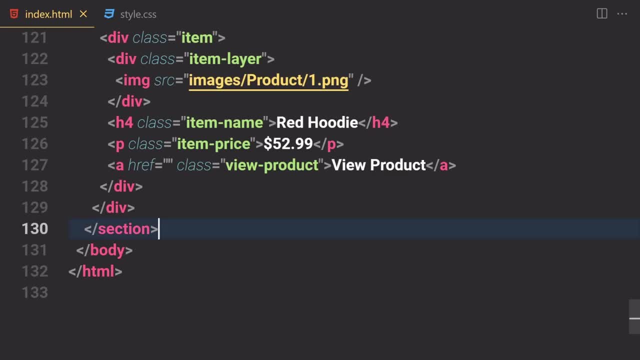 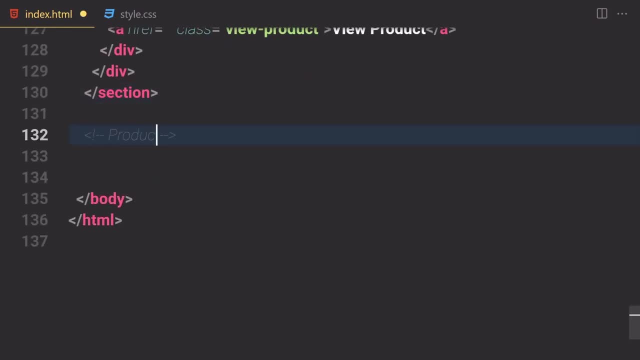 are not already done with this section as well. so what do we have to? what was the name of this section? uh, okay, so product section. we are not already done with our product section? let's just write products. uh, section end. and now let's just start working on this section. 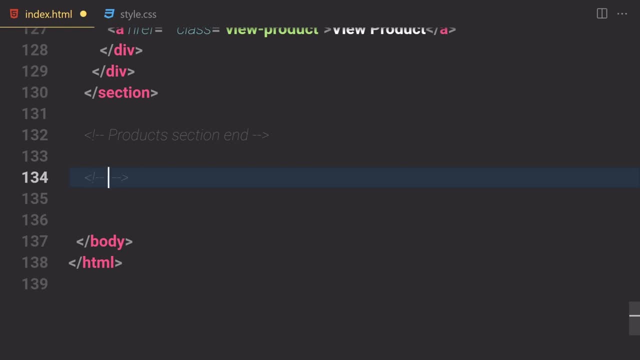 we are working on our new section, which is a customer reviews. so customer re c u s tumor uh reviews start yep, and we are going to be also writing an end for that inside there. we are going to be writing first of all our h1 with the class of customer uh heading. okay, so we are. 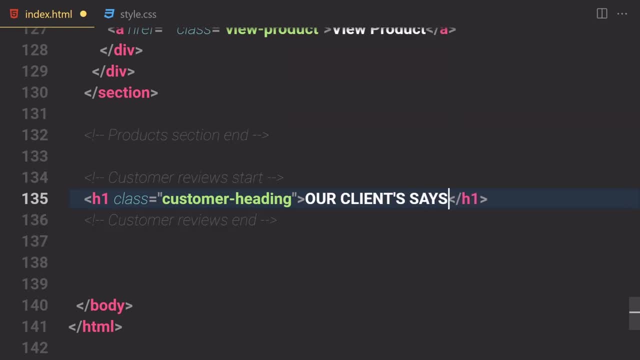 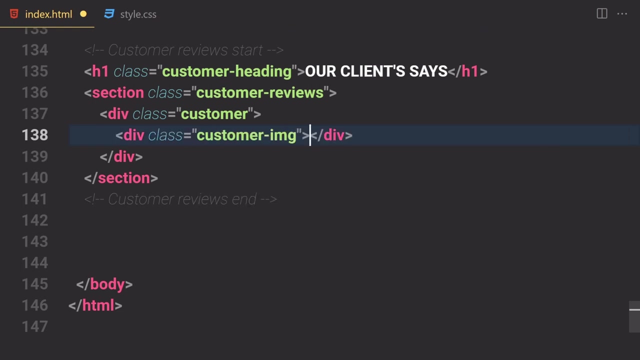 going to be writing, or clients says what section with the class of customer reviews, reviews, and inside there we are going to be writing a customer like so, and inside there we are going to first of all need a customer, uh, image, and then we would need image and then image one. 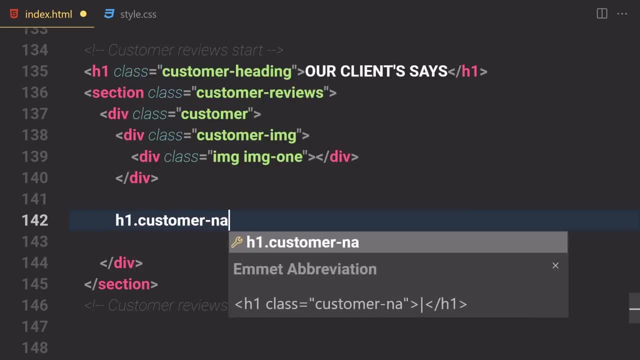 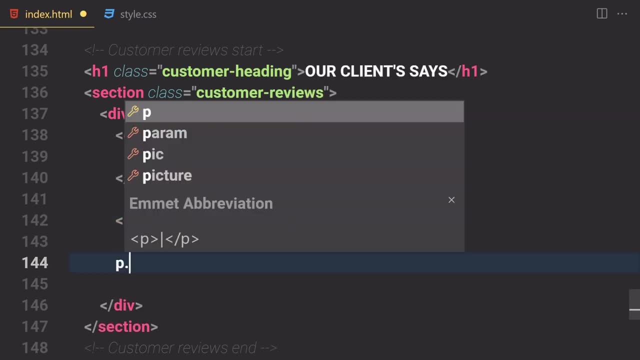 underneath this div, we are going to be writing h1 with the class of customer name. her name will be anna maria, and let's just write a paragraph for the class of customer description and let's just put a little bit of lorem ipsum inside there. i'm going to just go with the. 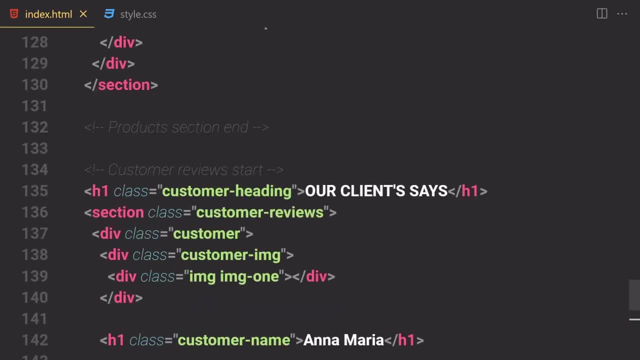 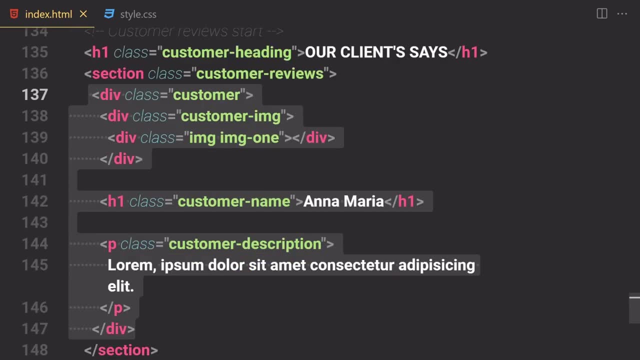 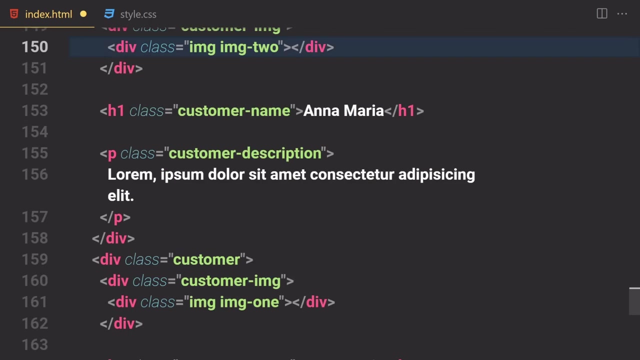 this elliott or elite, whatever you want to call that, and let's just duplicate this customer a few times. so we are going to be selecting that and we have our first customer and we have second and third. so, yep, the images are the same. so let's just use image two in this case and then to be 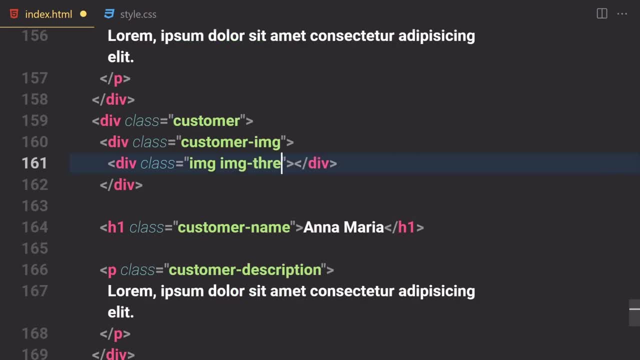 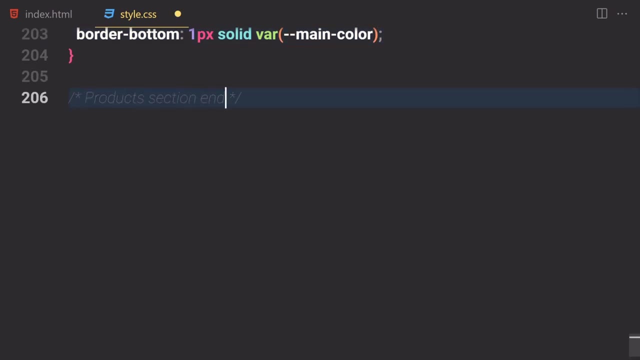 i don't know, let's just not worry about the name, so this one will be three. so customer and customer images. so if you sell that, we have all of these people's right here, but we don't have images. so let's just get into our css and write a comment like products section end and write uh. 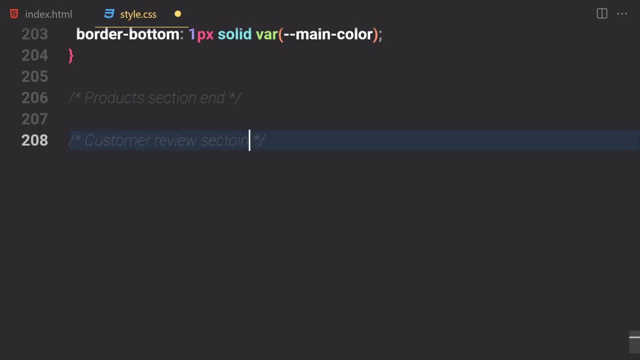 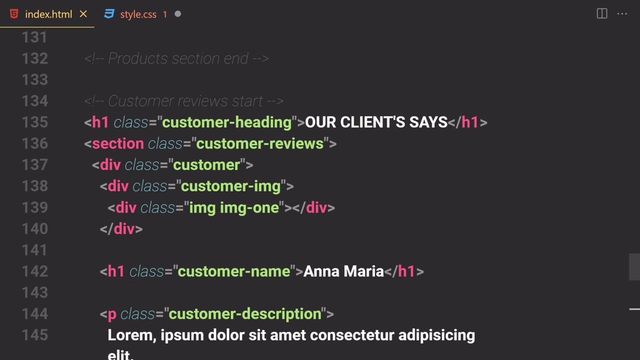 customer uh, review section: start, section: start uh, duplicate that and change that to end as well, and we're going to be placing all of our customer review styling in here. so, customer uh, okay, c-u-s-t-o reviews, just check the classes. so, customer heading, customer reviews. 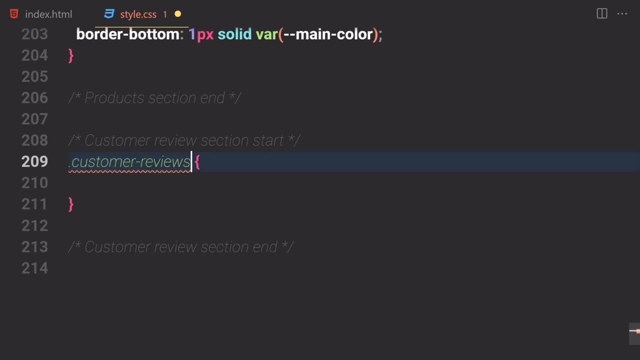 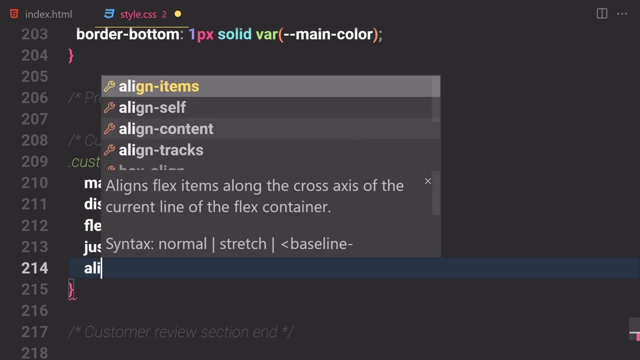 copy there. i'm not sure about my spelling, so i'm going to pass it in here. customer reviews. margin for the top will be five. frame display will be totally flex. flex wrap will be now set to wrap. justify content will be now set to not center but space around and align items will. 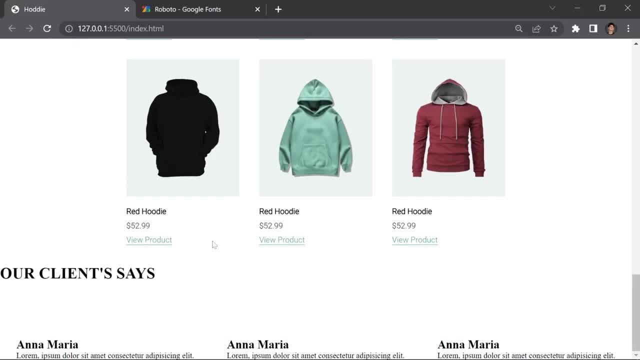 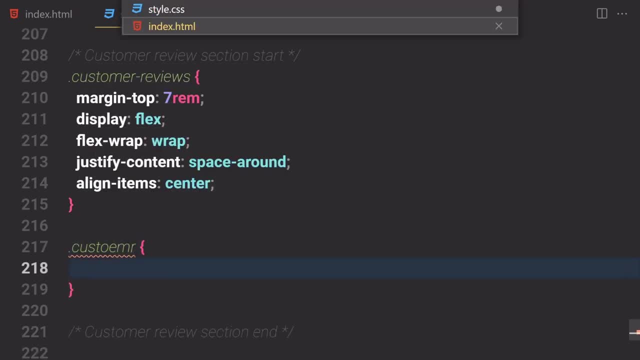 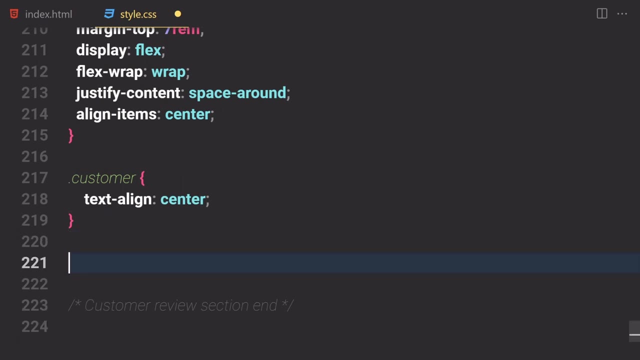 be set to center. okay, so that's it about their customers review. you cannot see that right now. let's just select for each customer: c-u-s-t-o-m. oh my goodness, i'm going to have to copy this name. yep, text align will be now set to totally at the center. let's just get or customer heading. so. 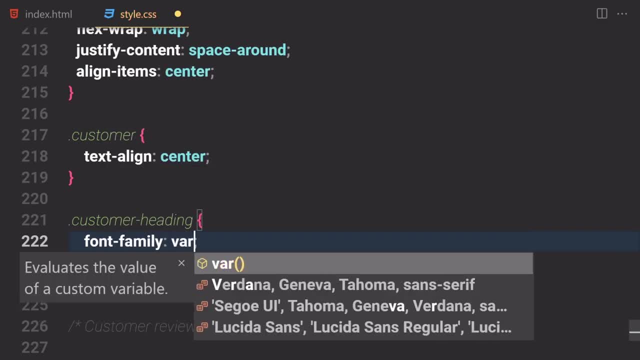 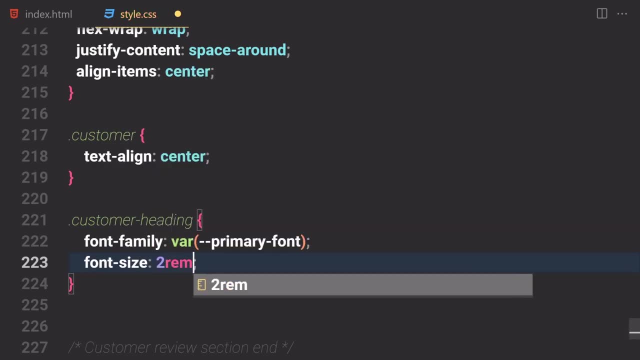 customer heading. okay, so font family will be now set to totally that main, not main, but primary font, which, if you, which you use as a variable font size, will be two ranks and the other level will be two rim and margin bottom. i'm going to give them like 20 pixel and text align, leaving also to center and 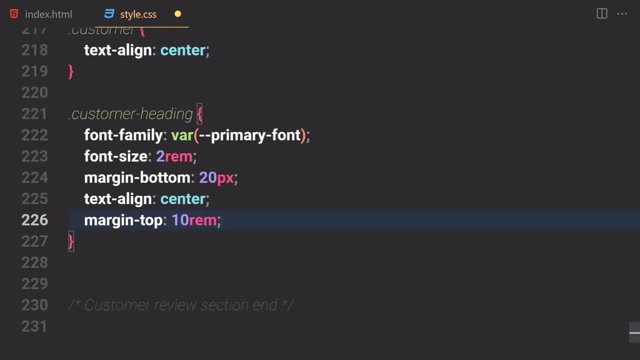 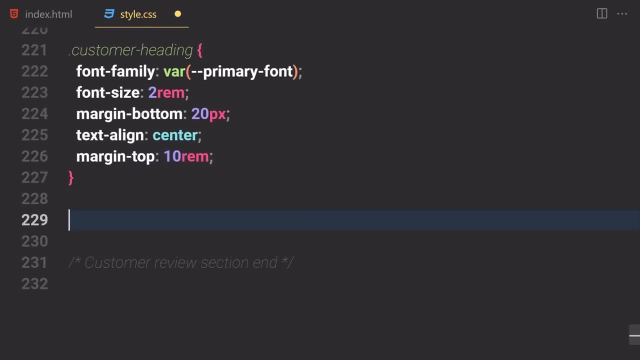 margin for the top area. i'm going to give them like 10 rims. so now, if you save that- and this is how it looks like right now, anyways. so now let's just start working on our customer reviews. so let's just use our customer reviews first of all, and then use a customer description. 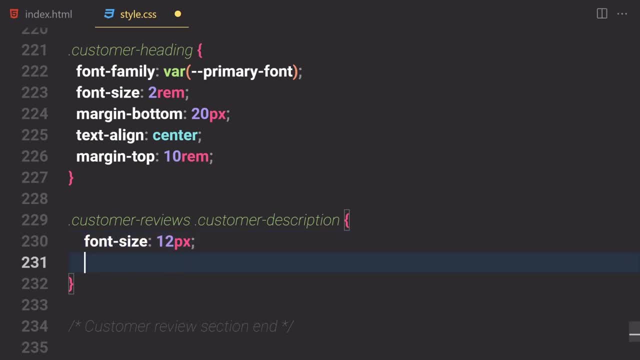 so font size i'm going to increase that to 12, not increase but decrease their 12 pixel margin. margin for the top will be 20 pixel and max width i'm going to give him like 200 pixel and text align in this case will be now set to center and margin i'm going to give. 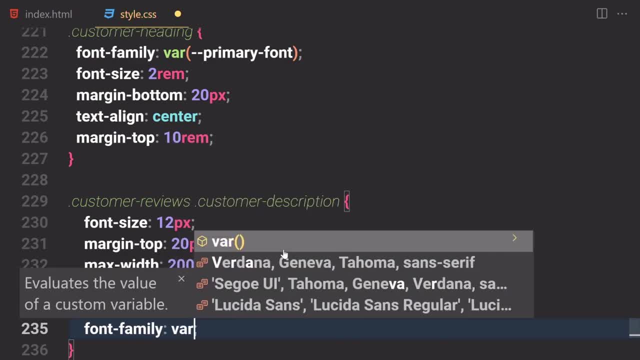 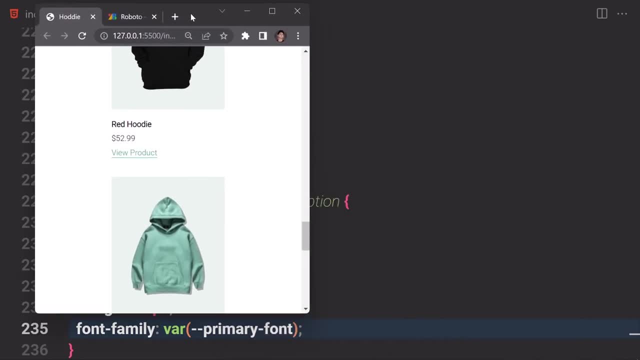 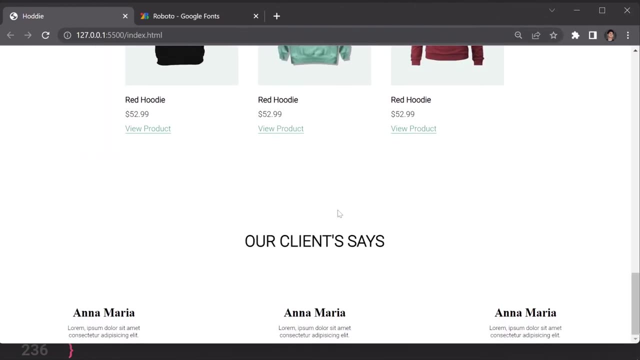 him is like 10 pixel. and finally, let's just use our font, family of war and primary font. see if you save that, and let's just make it a bit bigger so you guys can see everything. let's grab that in here. yeah, so now i guess that it's time to place our images in here. 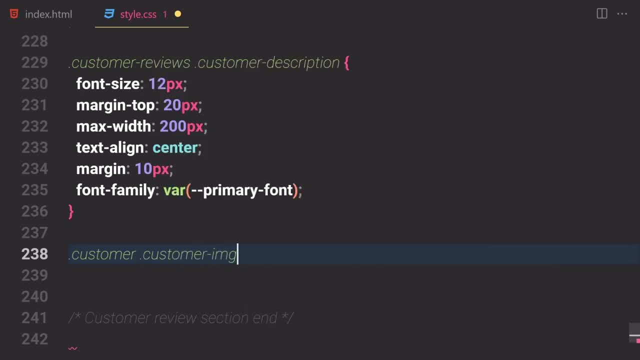 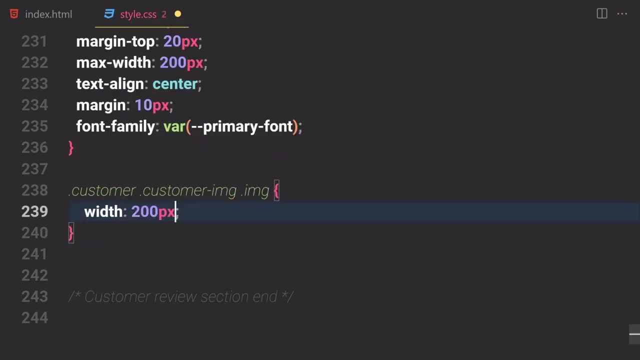 we have our customer and then we have a customer image, and now let's just get the image. so what do we have to do? we gotta give them a width of some sort like, uh, 200 pixel would be fine. duplicate that. oh, my goodness, my shift key is not working. i don't know why. 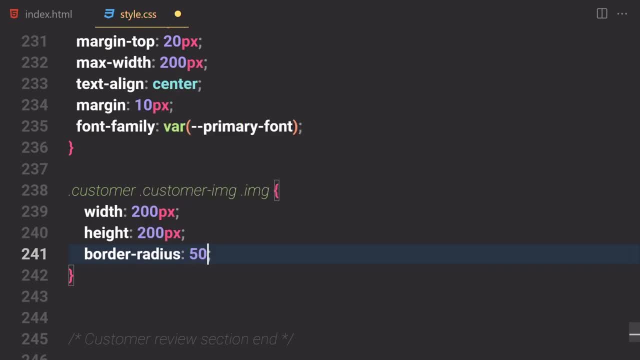 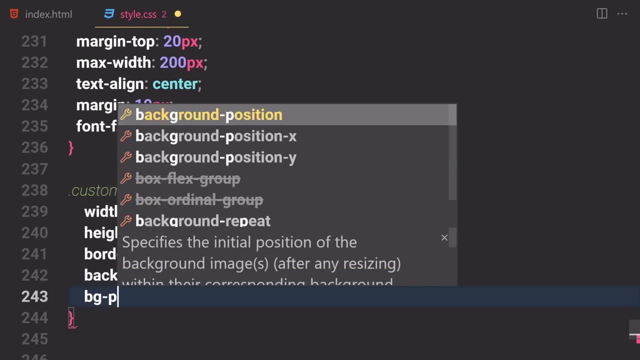 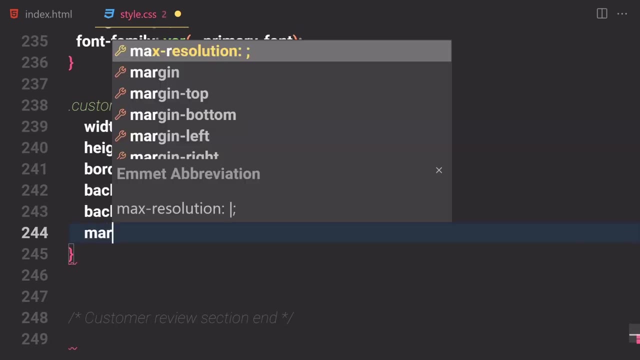 and then height, and then let's just provide a border radius for that- 100 percent. and background size we are going to be using is cover, and background position i'm going to give him is like center. background position will be now set to center and margin. i'm going 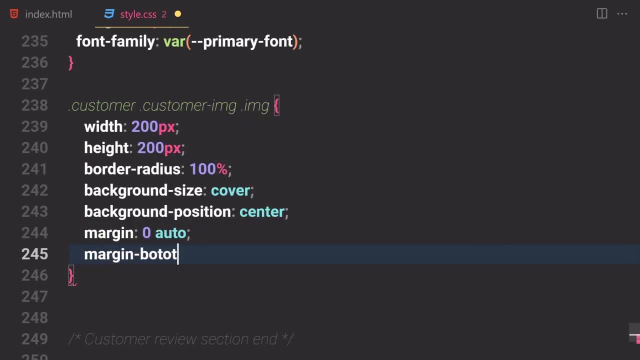 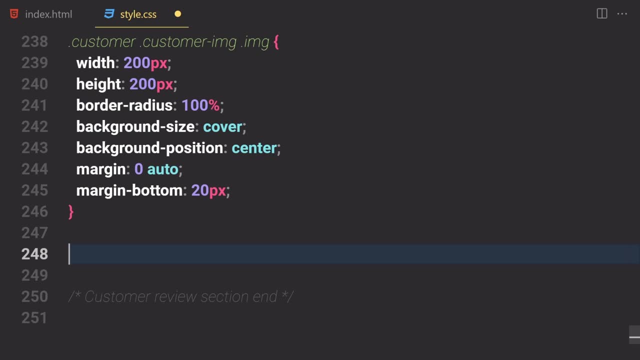 to write margin zero auto and margin bottom: uh b o double t o m of like 20 pixel. and now let's just use our images. so we have customer one, two and three. so we are going to be using customer, then image one. so what do we have to do? we have to just use a background image. 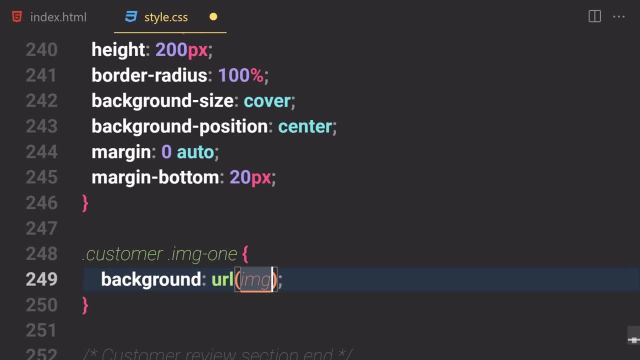 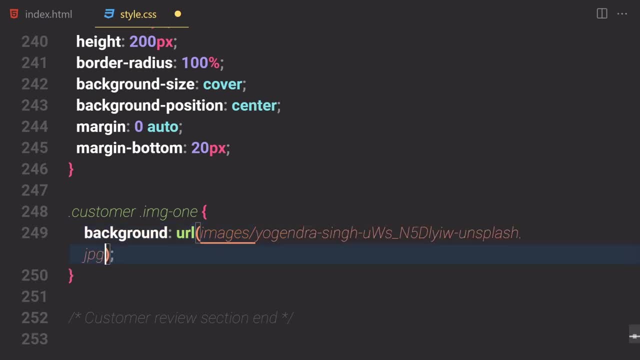 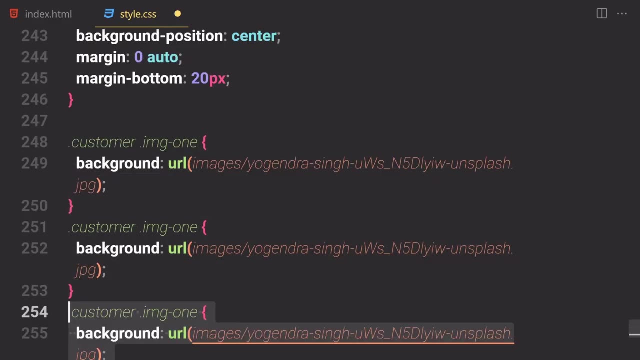 of url and let's get into our images folder, go back images folder. inside this images folder, we are going to be selecting, uh, this last one image, and now, if you save that, so here you can see, this image will now take its place right here. let's just duplicate that two times. so this is going. 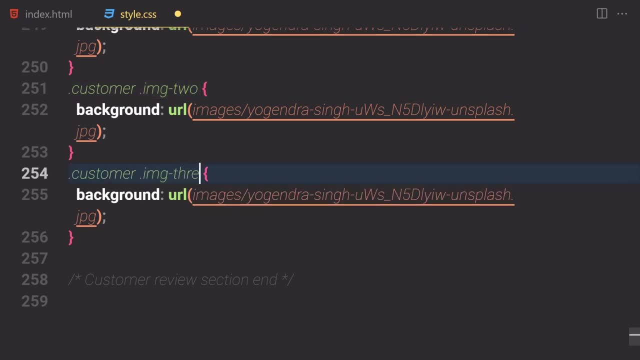 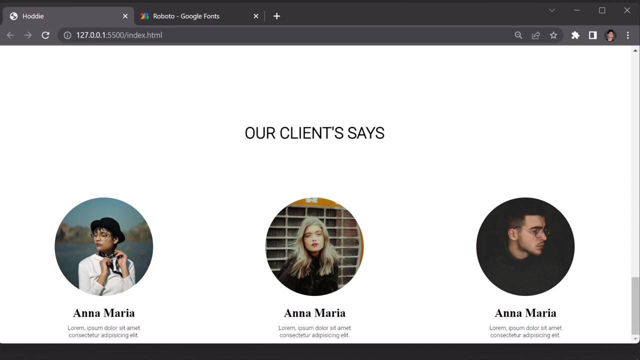 to be a customer two and this is going to be the customer three, and let's just change these images to something else, like this josh one and this one will be set to um million or whatever. so save it. and yeah, this shouldn't have to be an n, it should be like maybe some sort of a john doe. 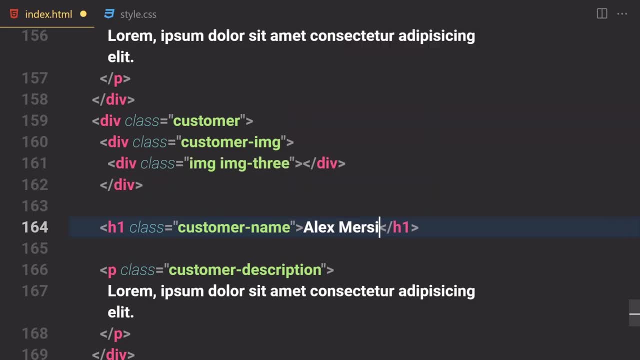 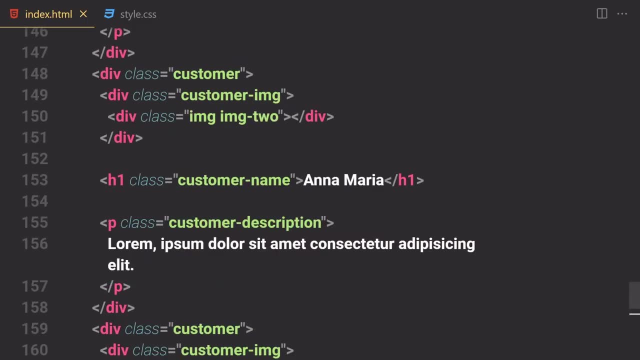 uh, alex would be fine, alex merson. so if you sell that, you have our alex merson. then we have our anna, and i don't know this is going. her name is going to be like: uh, alisa, maybe alisa, alisa, or yeah, at least i would be fine. so if you sell them, 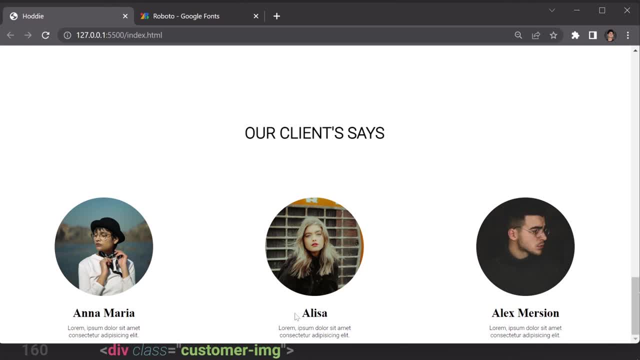 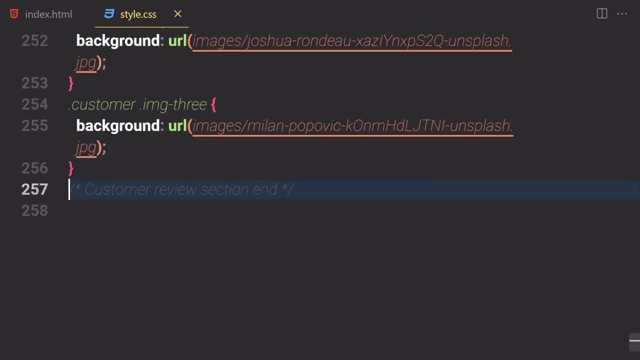 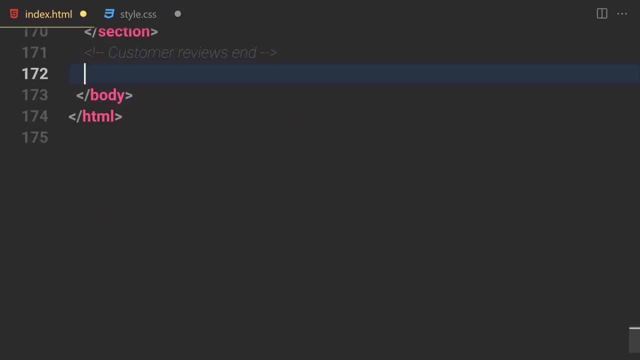 i'm not sure about this name, if there's a valid name or not, but i just give her name anyways. so that's it. yep, that's it about a customer review sections, and now let's just finally start working on our footer area. so this is going to be the final thing of our project. 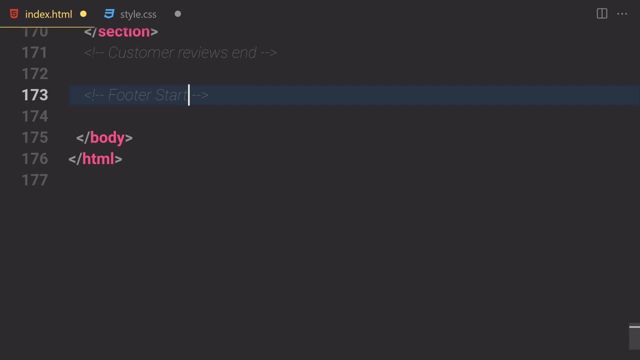 we are going to provide some footer content. so here we just have provided our photo. start and duplicate that for end. let's see what i wrote footer inside this photo we are going to be writing our container. inside the container we are going to be writing a further heading and 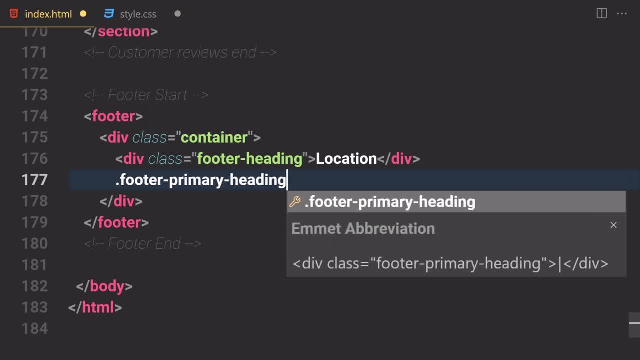 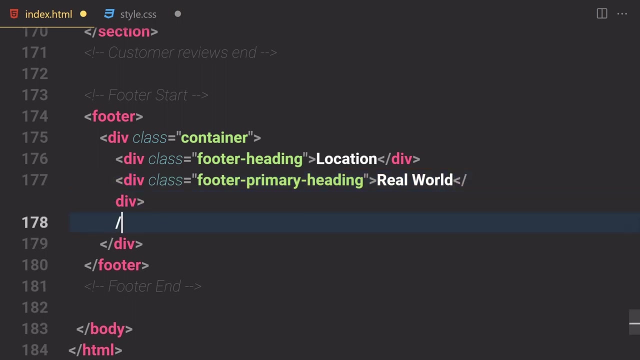 here. it will be now set to location and then we have a footer- uh, primary heading. okay, so we are going to be writing like a heading. i don't know, you can just go with any heading, like, fine, so if i just put like a real word in here and let's just write a street as well, so we have. 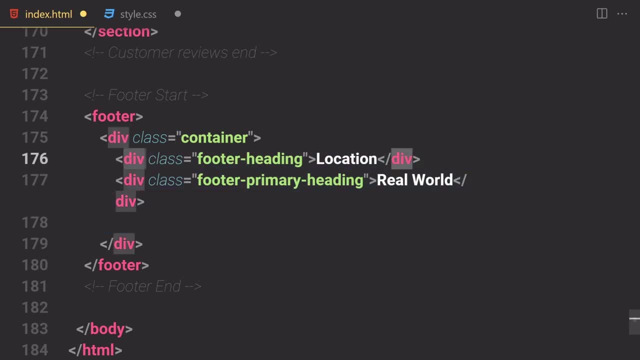 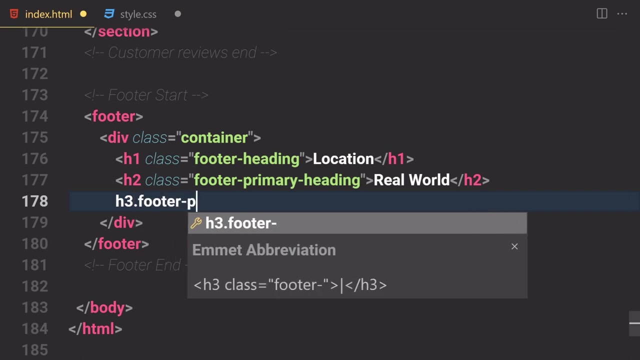 another footer. okay, so this is going to be our h1 and this one will be our h2. so now let's just change that to h2. h2 in here as well, and this one will be our h3. let me just get third button footer, primary headings as well. so we have primary heading, so we have four, two, one, three. 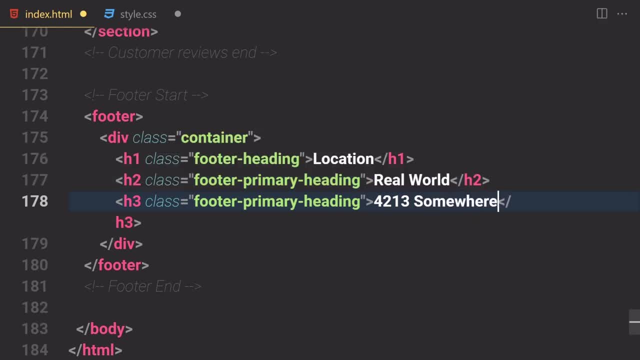 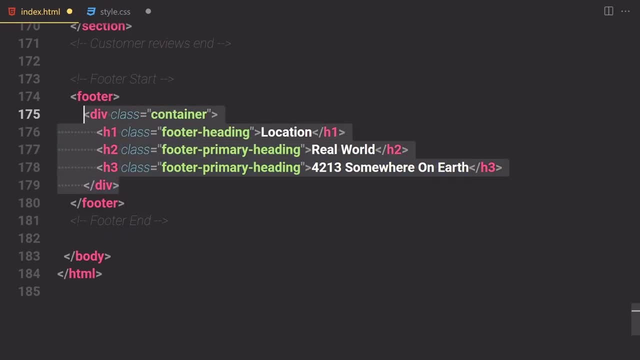 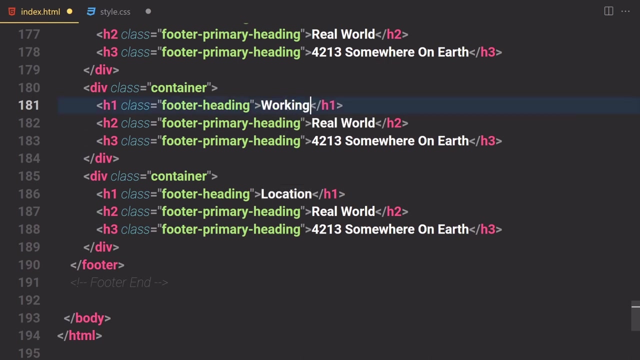 and this is going to be our street. some aware on earth back now. let's just duplicate that two times so we have a location. then we have like a working howards, so a working hards, and it will be like a working hards and it will be like a working hards and it will be like a 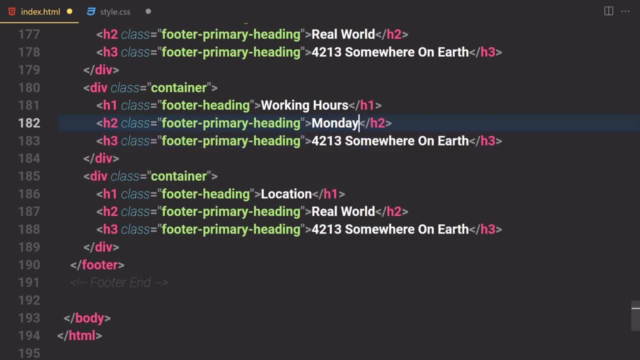 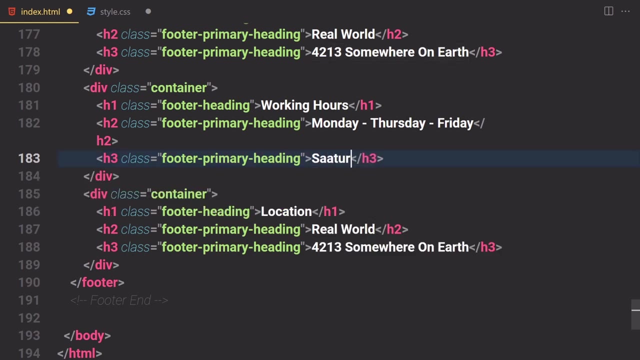 we now set to i don't know a monday, dash thursday, and also dash friday and saturn day. they're sunday and let's just change this one to contact us. uh, yep, that contact us would be fine, and i'm going to remove that and change it to contact us. 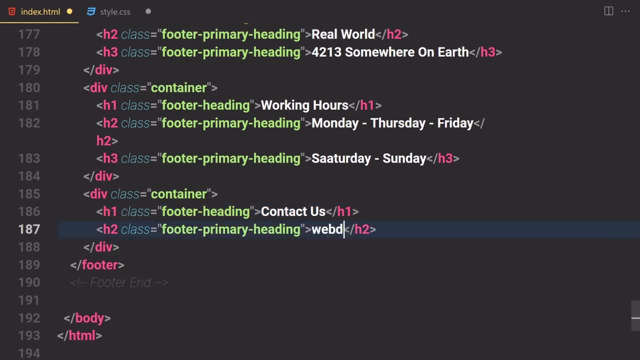 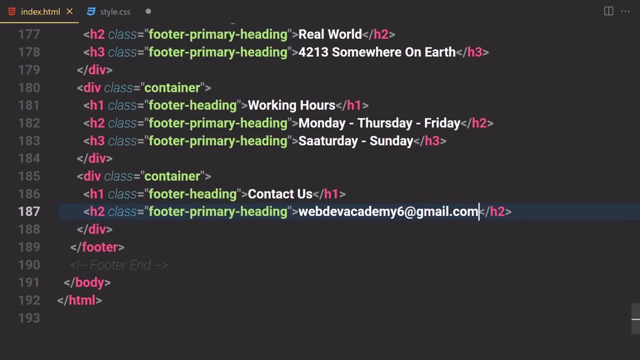 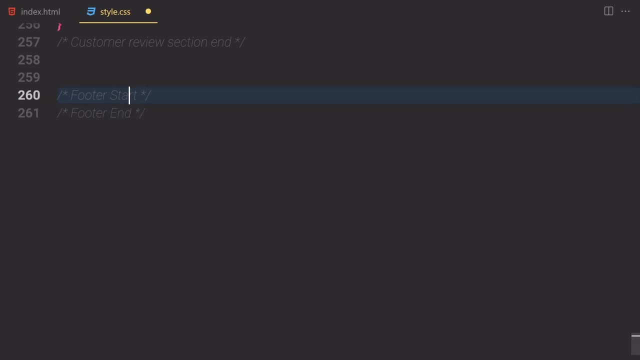 and change this one to my email. so web dev academy 6 and gmailcom. so if you save that and this is how the footer looks like. so now let's jump into our css and footer start and footer end. okay, so zoom in. let's just select our footer area right here and we are going to be. 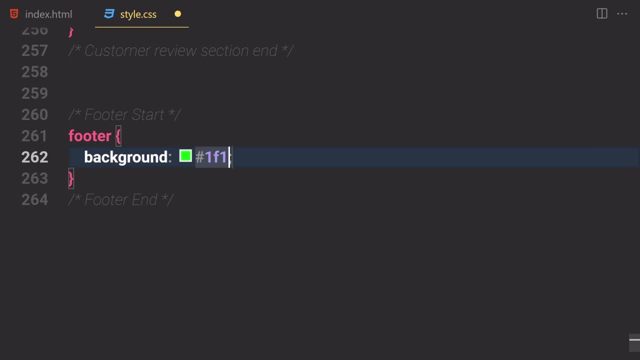 changing the background color to be like 1f1e- 1e one more time. so this is going to be the background color. let's just provide a margin top of 10 ram and the color will be totally white. and let's just use our display flex because we want everything to be wrapping, so for that we can. 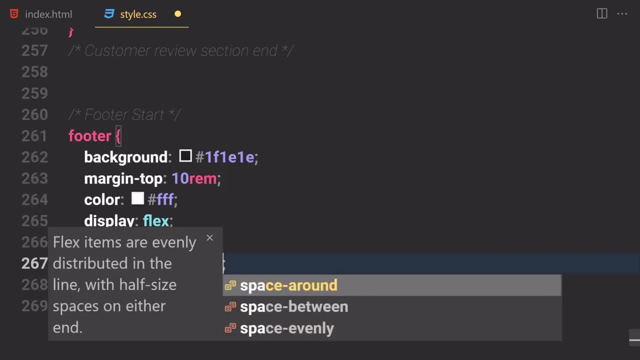 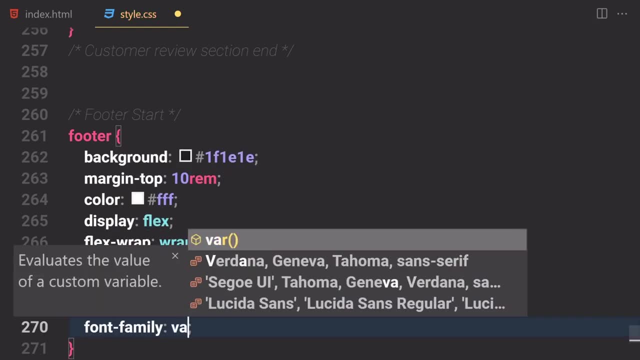 use a flex wrap of ramp. justify content will be also set to space around. align items will be now set to center and give them a height of 100 vh, and font family will be that one of our primary fonts. so if you save that and this is how it looks like, but now we have to tweak a little bit more. 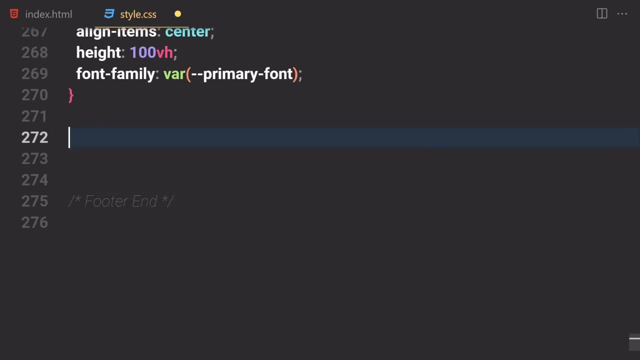 things in there. so let's just get over here and we are going to be changing the background color to be like 1f1e- 1e. one more time our footer, footer and then container. inside this container we want to get our footer heading. so what do we want to do with that? so we are going to be using like a margin bottom. 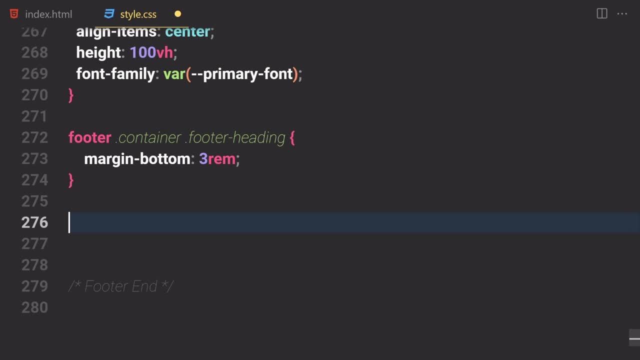 of maybe three rims. so let's just provide three rim and reuse. or footer. let's just provide our container and i forgot to get my footer heading. uh, not for heading, but for a primary heading. the font weight will be now set to totally normal font size i'm going to be using is 15 pixel and the margin bottom will be now set to 20 pixels. so 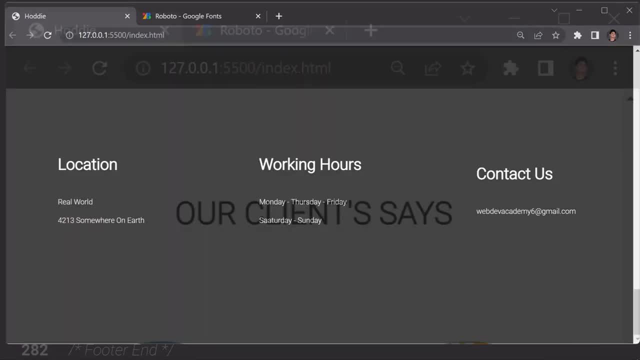 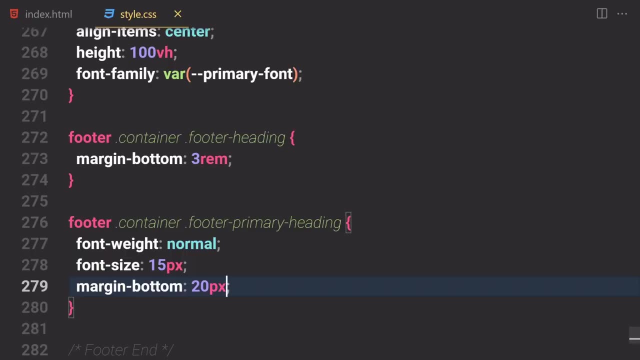 if you save that and this is how it looks like, okay. so if you just make it smaller, i know everything is looking weird because we're going to use any media queries for that. so now let's just use our media queries and- and this is going to be the end of our project- so let's just use 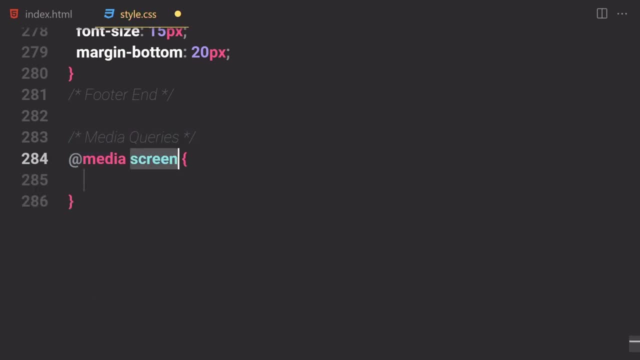 like a media queries. i'm going to add media for uh, only the screen size and also the max width will be set to 900 pixel. okay, so what do we have to do? we have to just write a header area, the height. i'm going to give him like 120 viewport height. 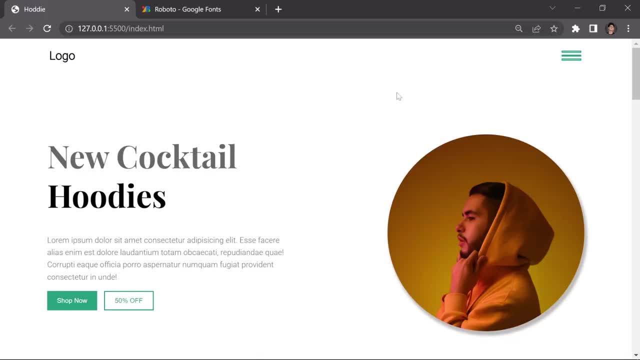 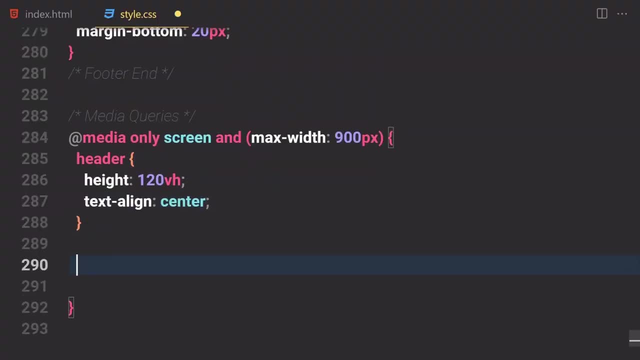 text line will be now set to center. so if you save that, make it smaller and this is how it looks like on a smaller screen sizes all right. so now let's just get or section one, uh, and we are going to be writing a section one, and height will be now set to like 120 viewport height and 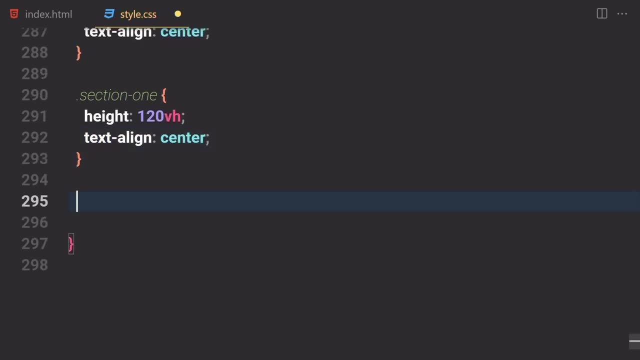 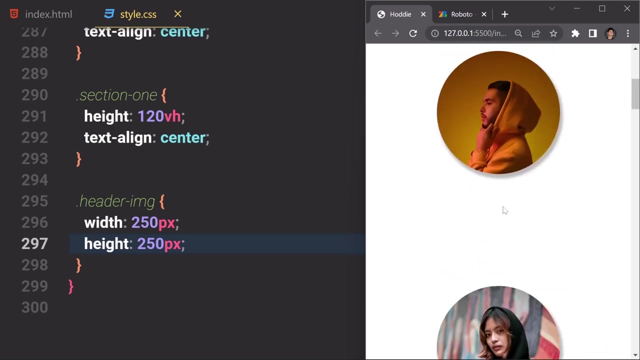 we also set to center as well. okay, so let's just get our header image. so i'm going to write header img and width will be now set to like 250 pixel and height will be also set to like 250 pixels if you save there. so it will now just uh, decrease the size of both of these images right here. 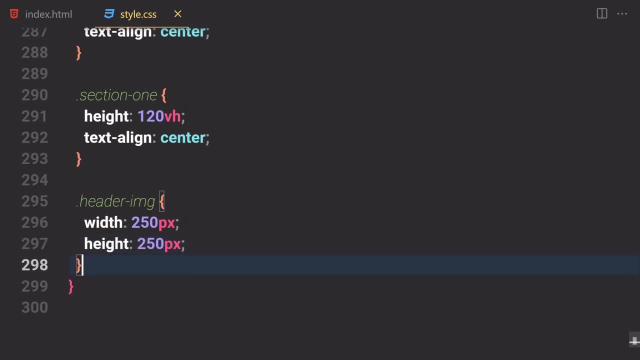 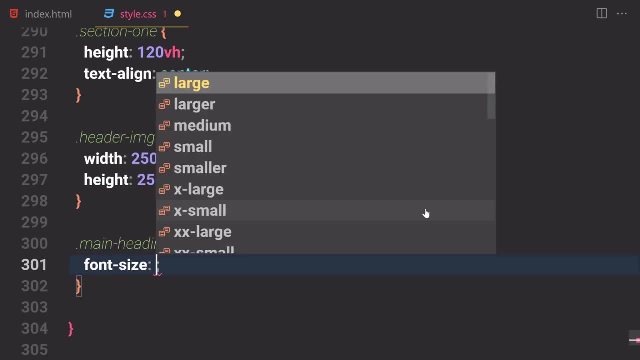 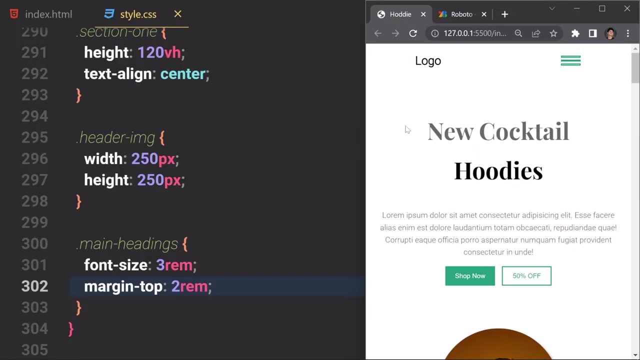 okay, so we are now totally cool with this section and now let's just try it, or let's just work on our main headings real quick. so we have our main headings and font size i'm going to be using is three rem and margin top i'm going to be using is like two rem. so if you save that and yep, that's. 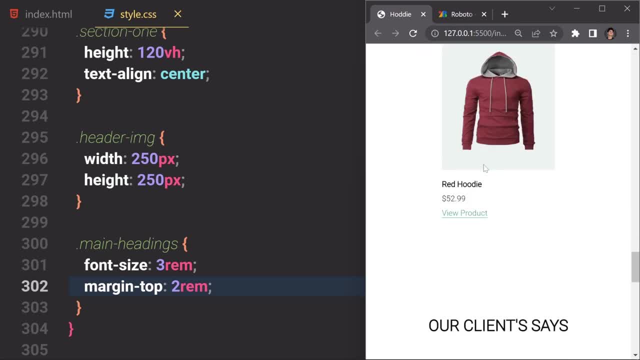 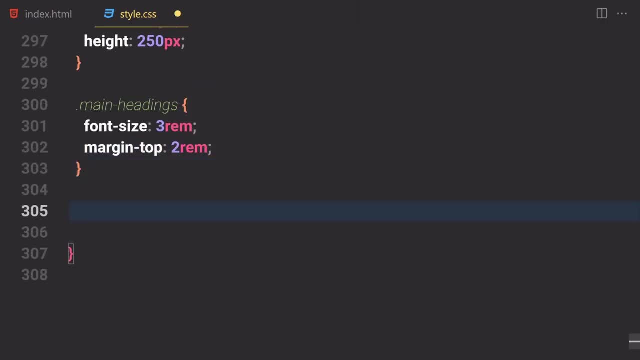 about our headings like main headings. so now let's just take care of our primary headings. which are these primary headings? so let's just take care of that real quick. so what do we have to do? we have to just write a primary headings and the width will be just 400 pixels. so if you save that and 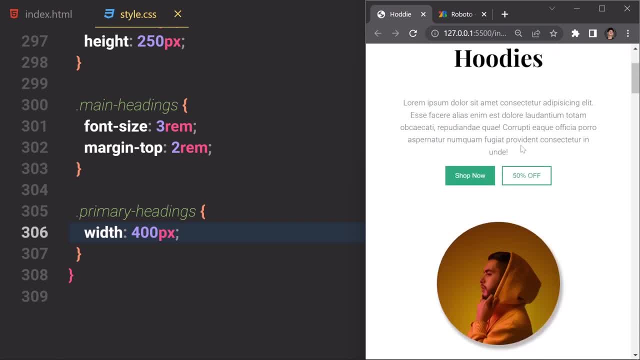 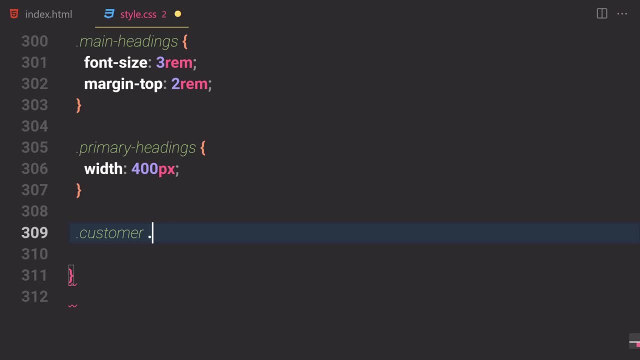 yep, that's looking a bit better and these are also looking better. so final thing which you have to do for this project is to just select our customer and select all of the customer images and select our image. let's just decrease the sizes of them, like 100 pixel width and 100 pixel height. so if 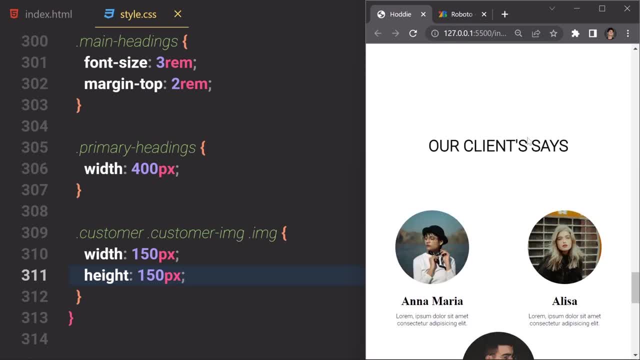 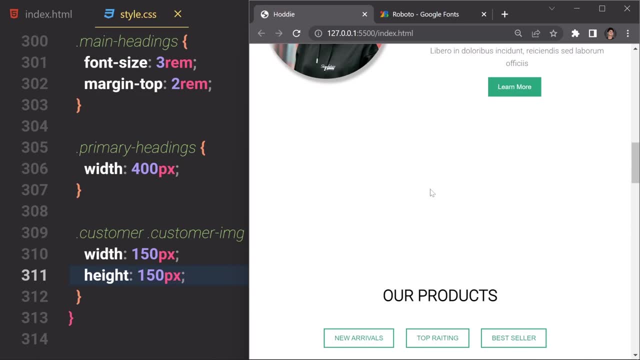 you save that and check them out. so this is how it will look like and everything is working the way we expect them to work. i'm going to make that just a little bit bigger, and this is how everything looks like. so if you just see that in a bigger screen, this is how it will looks like. 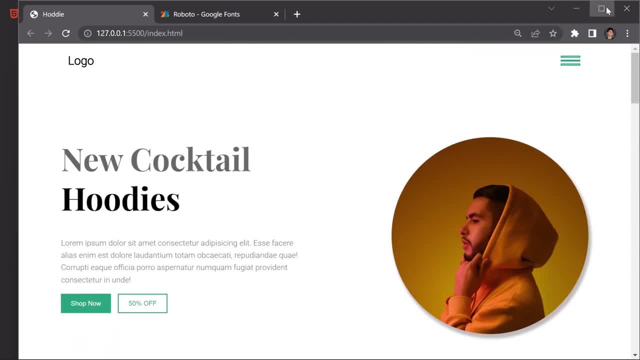 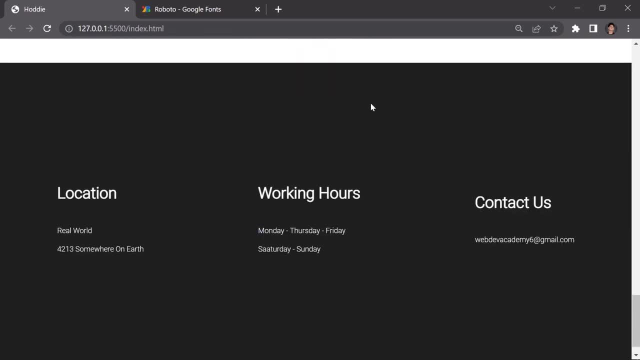 on a bigger screen. so if you want to provide a lot of styling, so this project is now yours. if you want to find the coding, so you will find the link in the description below. you can click on there and you can grab the code from there. anyway, so thanks for watching and i'll see you. 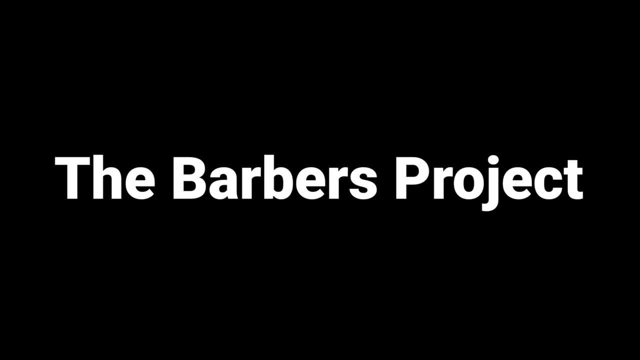 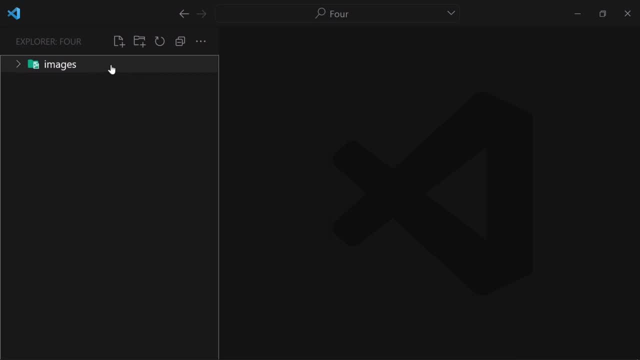 in the next project. all right, so before getting into the project, first of all i want to mention one thing: if you want to use the same images which i'm going to be using in this project, so i'm going to give you the link in the description below. you just have to click on. 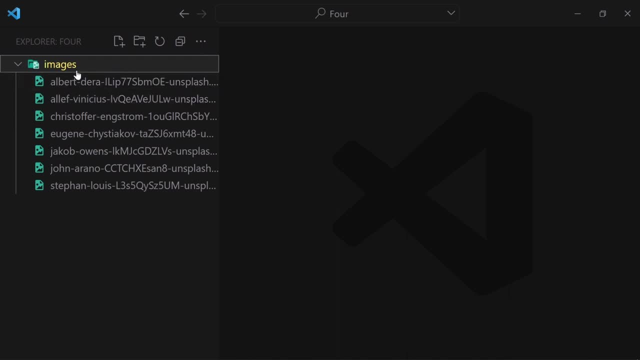 there and it will bring you to my github repository and you can download all of the code for this project and all of these images which i'm going to be using throughout this project, and if you want to use your own images, so feel free to do that. so now let's just begin by writing some code. 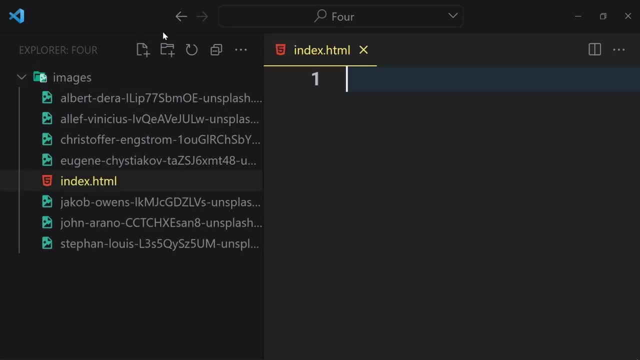 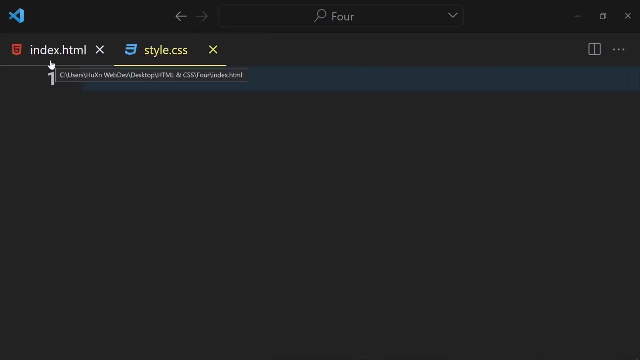 so, first of all, i'm going to just create a folder given name of like indexhtml, and i'm going to just drag it to the root, and now let's create a new file given name of like stylecss, and we are good to go. so now let's just write our doc type html in here and, yeah, that's going to be a. 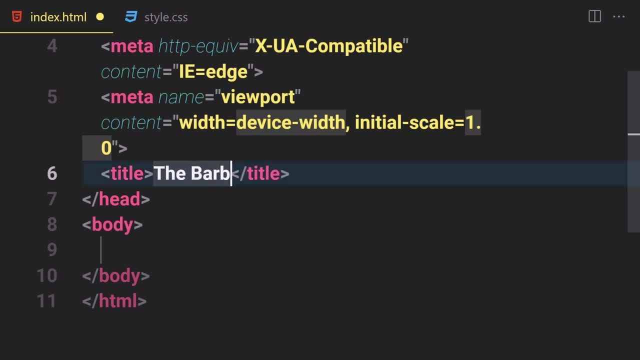 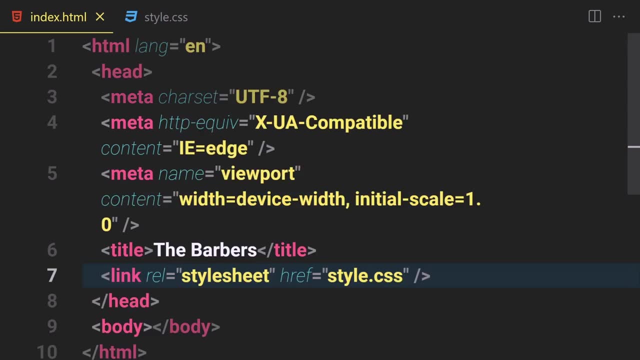 line, and i'm going to just change the name to the bar birds, i guess. so now let's just link it with our css file as well. okay, so now let's just link there real quickly, and i'm going to just hide this head area from there. right click on it and open it for the live server, and now we can see everything. 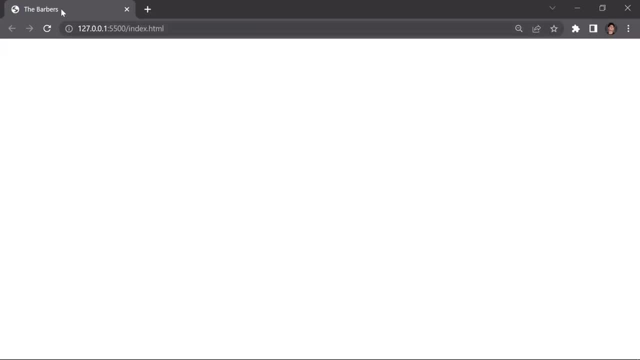 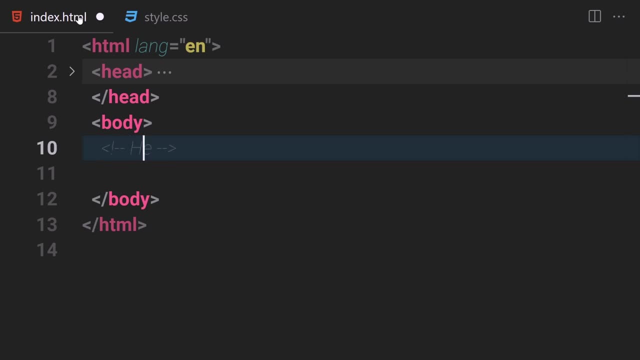 a bit clear. so it will open our file in a live server right here, and here you can see the title. all right, so that was the first thing. now the next thing which you have to do is for html. we are going to be writing our header area. so if you want to work with the header, 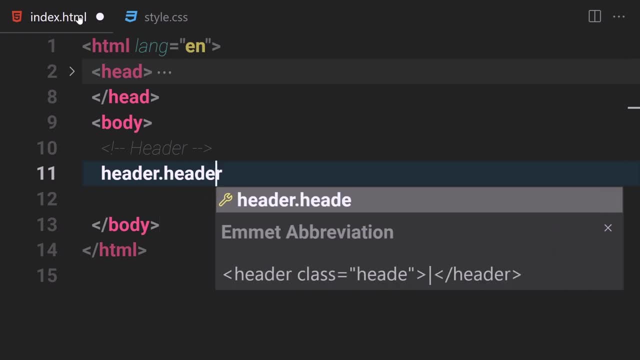 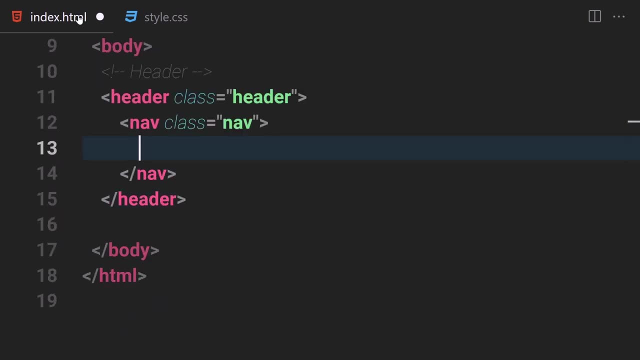 area. so we are going to be first of all writing a header and we are going to be also giving a class of header. so inside this header, we are going to be using our navigation and i'm going to also give a class of navigation. so inside this navigation, we are going to be writing h1 with 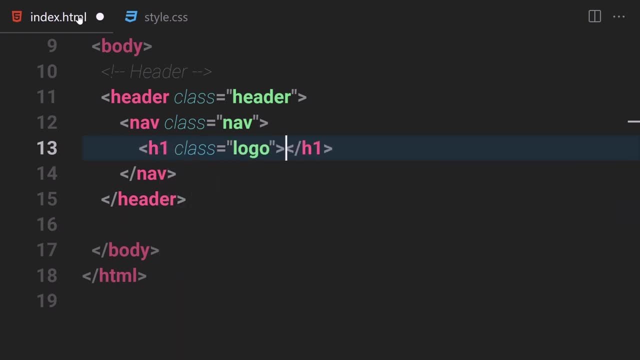 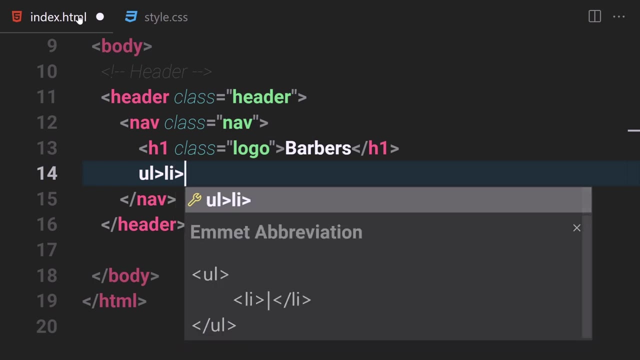 a class of logo. so just write a logo and i want to just put like bar birds inside there underneath this h1. we are going to be using ul and then li and then anchor tag, and we want that to be like: uh, i don't know four of them, so i'm going to just write four. it will go to nowhere. 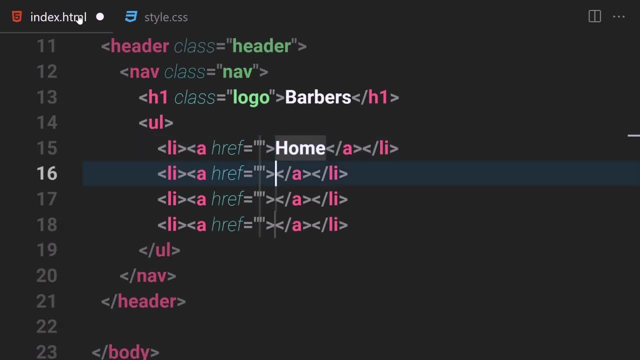 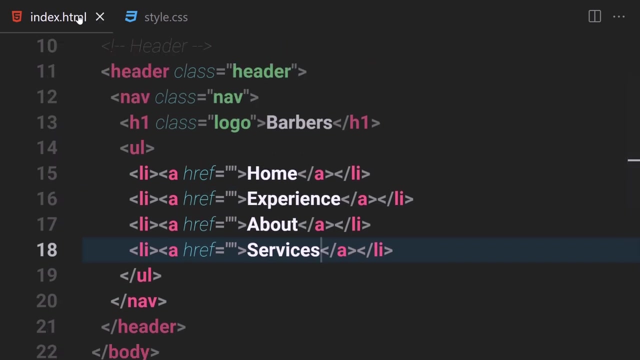 the first one we have is a home. the second one we have is experience, so experience. and now the third one we have is about section, and the fourth one we have is a services, services like. so all right, so now we are totally done with this header and navigation area. so now, if you save our file, 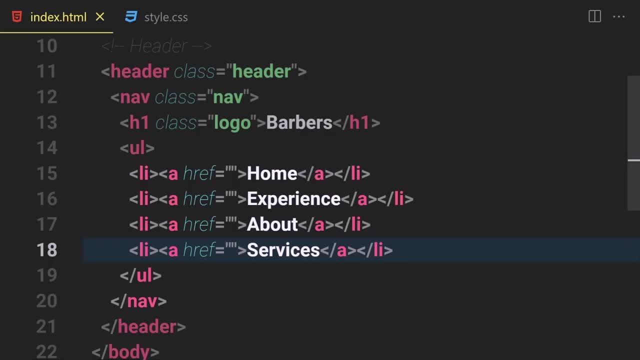 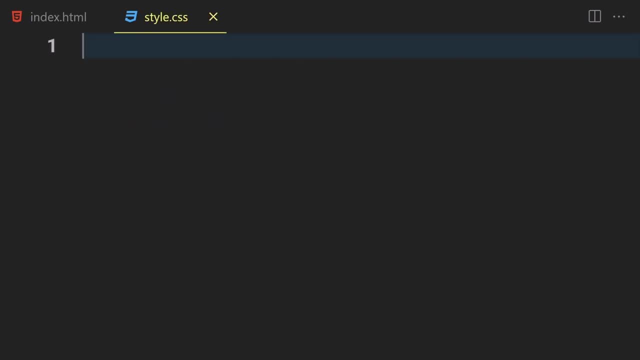 and this is how it looks like right now. okay, so i'm going to just zoom in a bit. all right, so we are totally done with the header html. so now let's get into our css, and now let's just style that. but before we do, first of all let's get into our css and let's just style that, and let's just 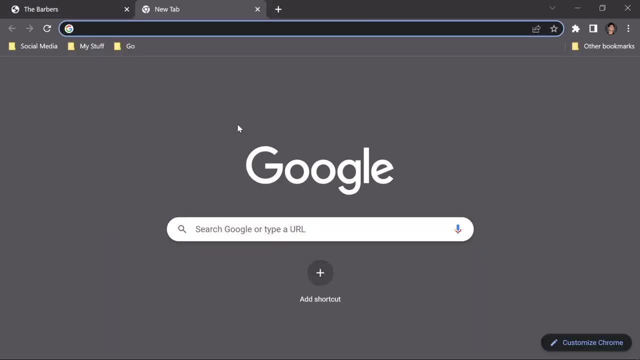 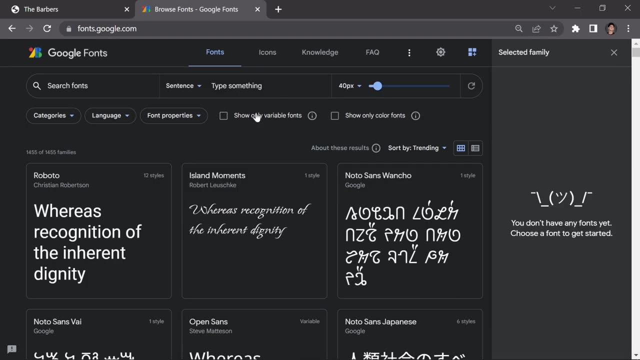 style that and let's just do a couple of things we need to do first of all. so first of all, we need a few things. so let's just get a fonts first of all. so i'm going to just write like fontsgooglecom, and here we are going to be grabbing two fonts, so i'm going to remove both of them and let's just 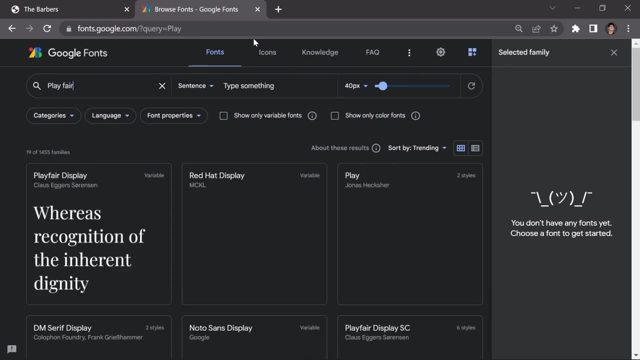 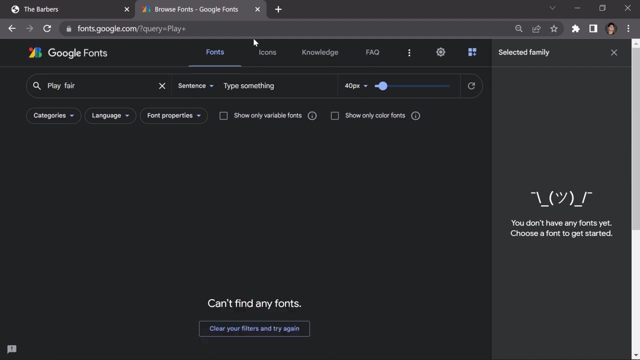 search for the first one, which is that play, uh, fire or fare whatever you want to call it f-a-i-r. okay, so i just messed it up something and i'm not sure. okay, so fire display: is that a fire or fair? let's just see bear display, yep. 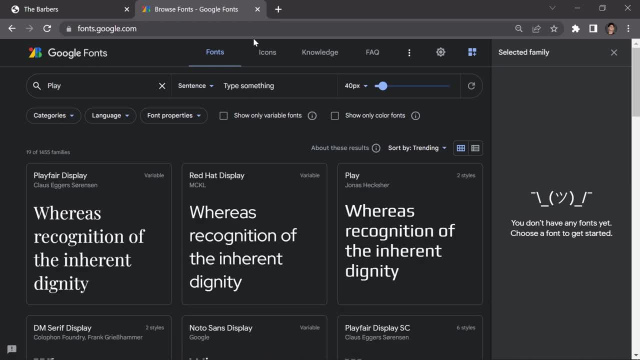 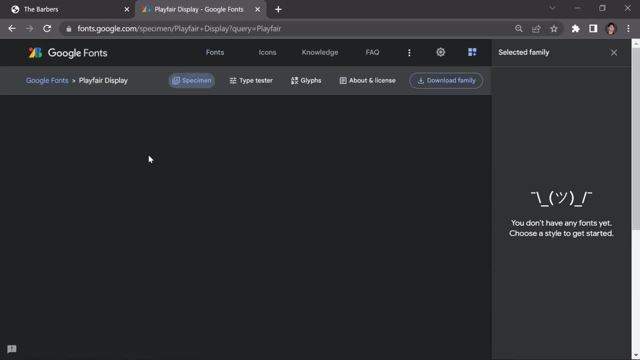 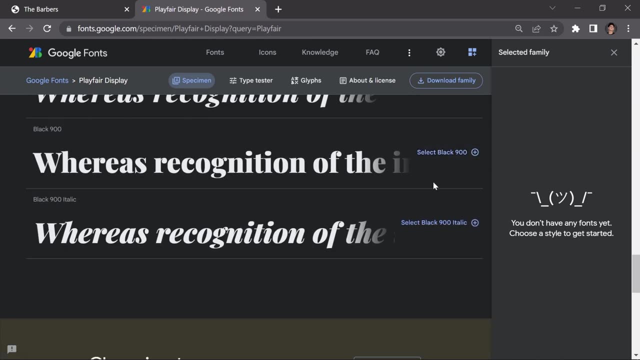 okay, so it's not giving me any hints of play. and if okay, so let's just write it manually, like so? all right, so now let's just select the second one, i mean like the first one, and we would need the weight of like eight, not 800, but 900 would be fine. we want a huge, bold one. so i'm going to 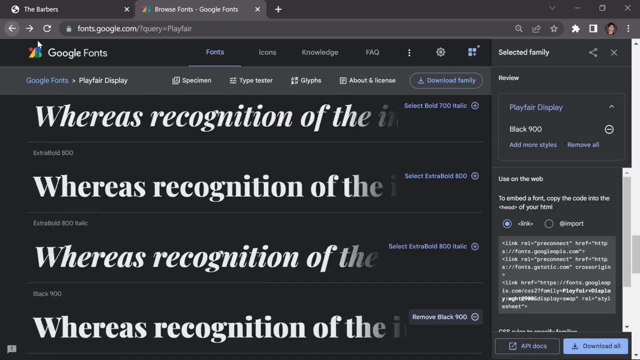 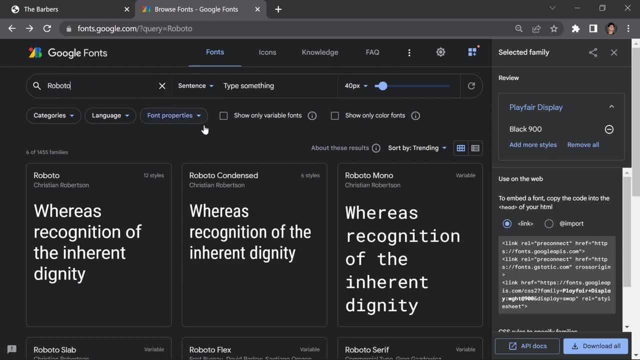 just click on this 900 font weight and now i'm going to just go back and now let's just search for a font color: roboto. so i'm going to just search for roboto, like here, and i guess we're not going to be using that roboto that much, but we will just grab it anyways, and i'm not sure about 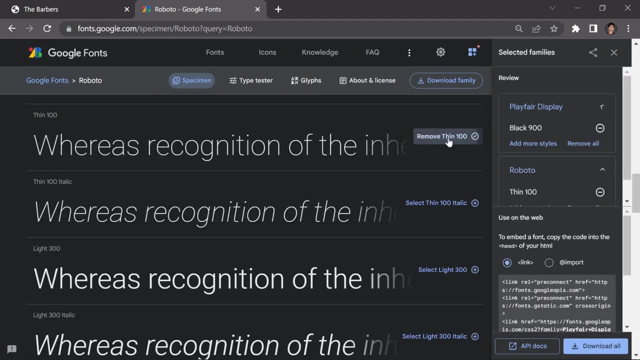 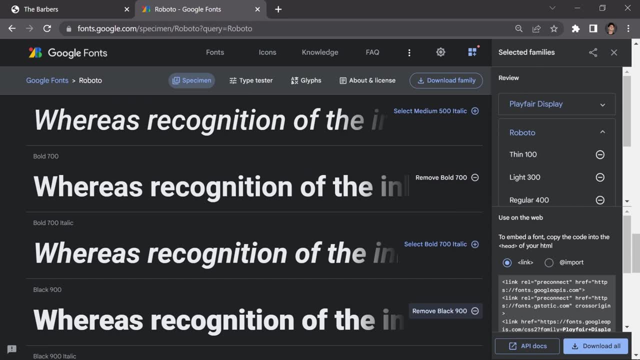 the font weight of there. so i'm going to just like grab all of these fonts, so 300 regulars, one, not italic one. so we are going to be selecting all of them, all right? so now we are totally good to go. so let's just click on this import and copy that. so i'm going to copy that and i'm going to. 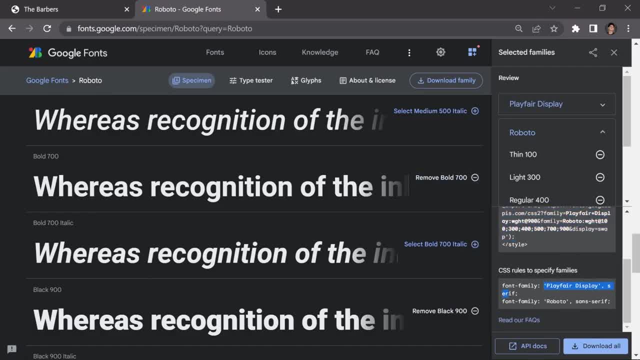 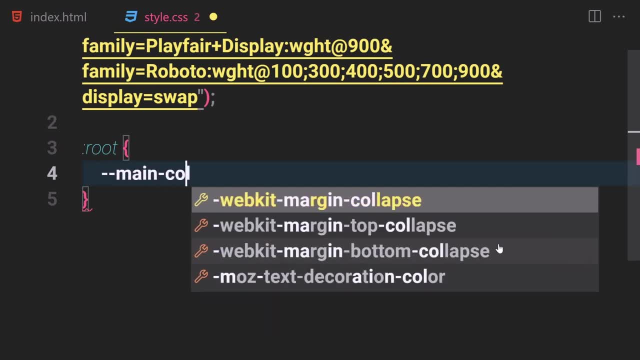 paste it right here and also let's just grab there. and now let's just create a variable first of all. so we are going to be writing a root and then just write a main color, or you know what? we are going to be writing main color just in a second. so first of all, just write a main um font. so i'm going to 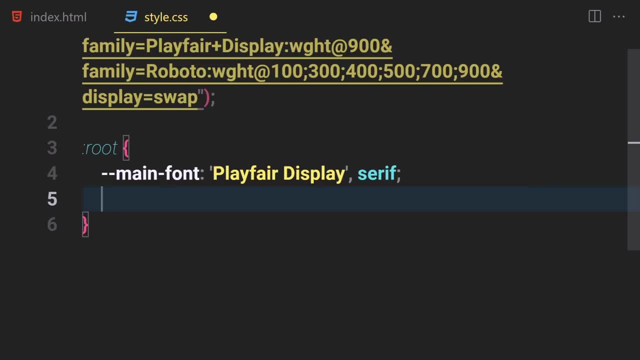 just place this, play fire or play fair, whatever you want to call it. i'm going to create a new variable given name of, like secondary font, or you can also call it um, custom, custom values, or whatever, and i'm going to now put these uh font value in here and now. let's just create a variable. 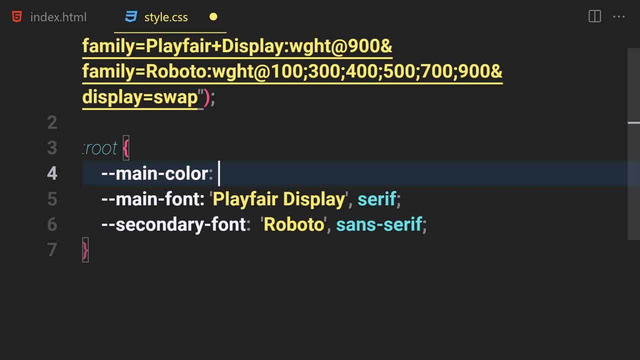 for our main color. so we are going to be using this main color like 37- oh, my goodness, 3713- and 2d. i guess this is going to be the color which you are going to be using throughout. if you want to choose your own color, so feel free to do that. and now let's just 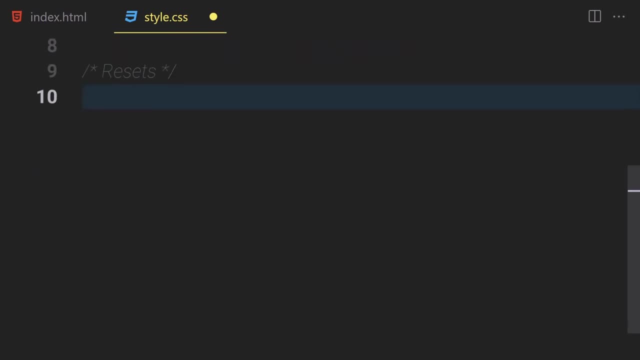 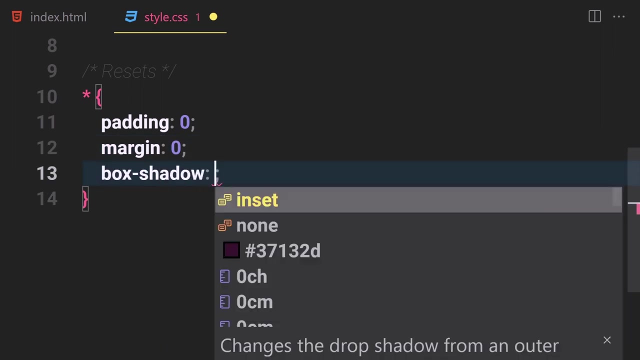 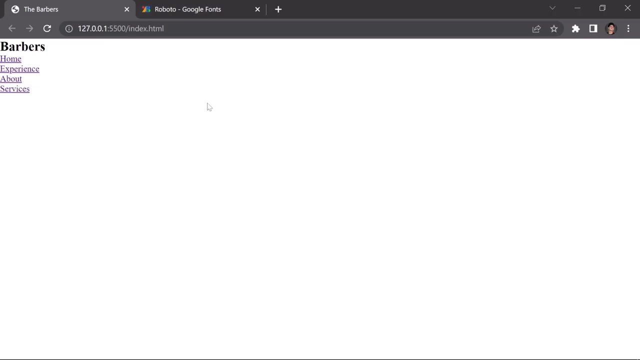 write or reset. so here we are going to be just placing or reset. so we are going to be starting from: uh, padding will be totally zero, margin will be also zero and box sizing- not box shadow, but box sizing- will be border box- all right. so now, if you save a file, so currently things looks like this: 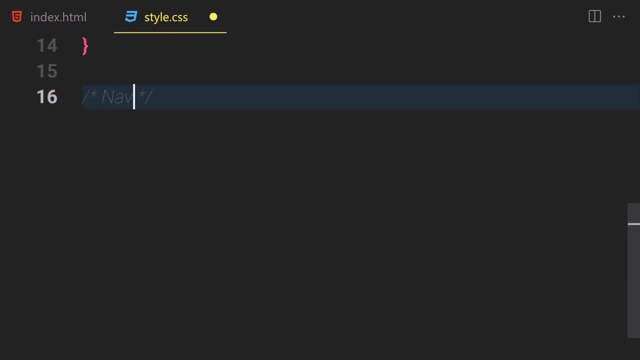 so now let's just start working on our navigation. so i'm going to just write like a nav in here, or you know what nav star would be fine. so if you just write, so this is going to be your nav star, and then we are going to have our nav, and so let's just start working on our navigation. 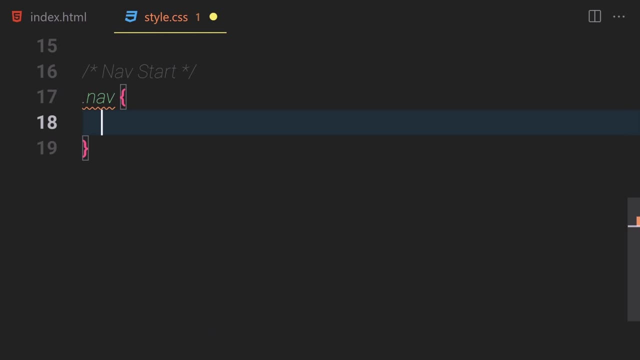 so we just select this nav by using our class right here and we are going to be using a display of flags: justify content will be spaced around because we want a little bit of spacing around that item. so we are going to be writing: align items. it will be now set to totally center, so 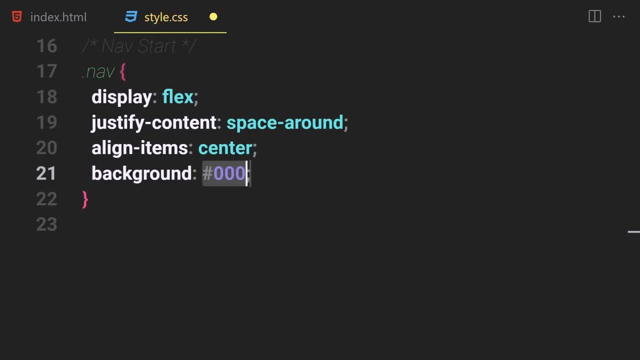 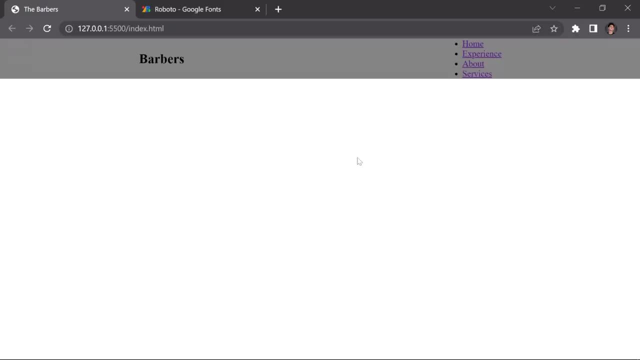 and this is how currently things looks like. so if you just provide a background color of black and if it's several file, and this is how it looks like, or you know what you're going to be making that a little bit of subtle like, so so save it. yep, that's looking awful, i know. so now let's just 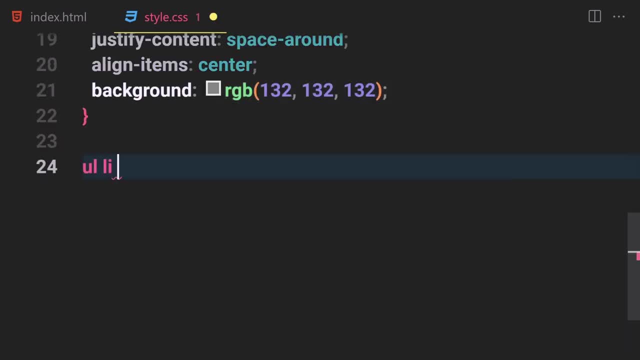 use that ul and li. so we are going to be selecting this ul and li and which is this ul? and inside this url, we're going to be selecting all of these allies. so now let's just select that. and what do we have to do? first of all, we want to remove that list tile from there and also we want to. 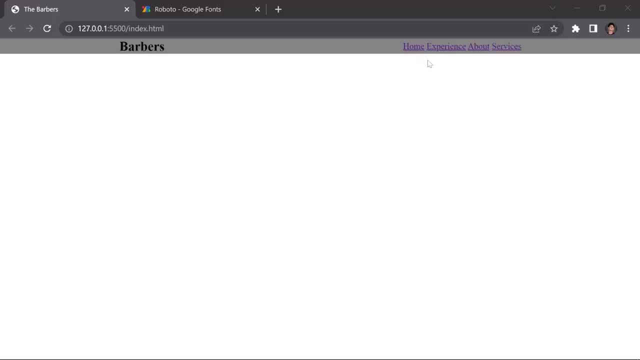 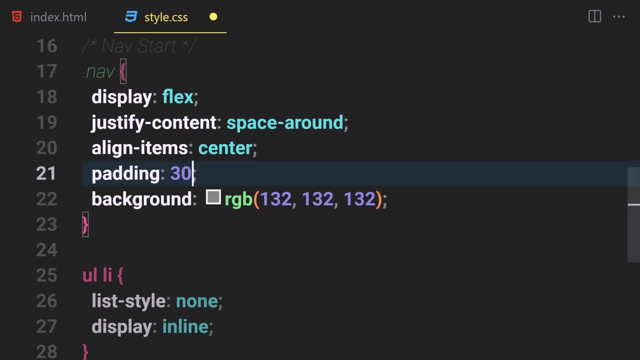 use a display of inline. so if you save that and this is how it looks like right now, okay, so we have to provide a little bit of spacing or padding in there. so we are going to be using padding of like i don't know, 30 pixel will be fine, so let's just check this out. if you save that, yeah, that's. 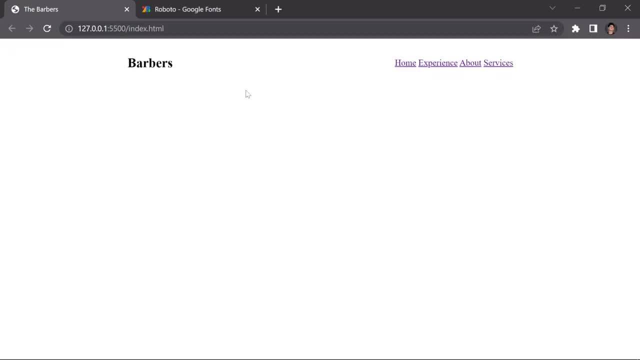 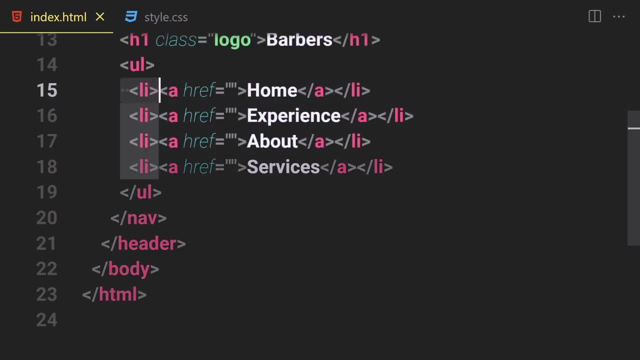 cool. so now we have to remove this background from now and this is looking better, all right, so now let's just style: uh, these anchor tags right here. so all of these anchor tags which is inside each of these align right here. okay, so we have to first of all select a ul. 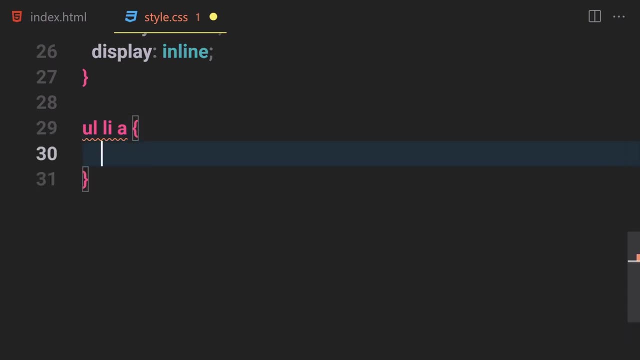 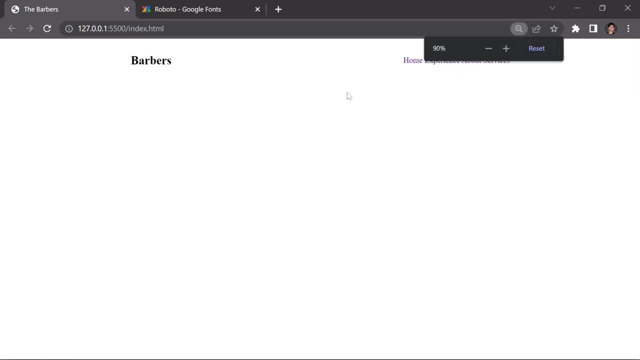 inside the ul and then select or anchor tag. and now let's just select that and use a text declaration of none. so if you just save that and here you can see, it will now remove that uh ugly kind of border or line, whatever you want to call it. so we'll now remove that. now let's just provide. 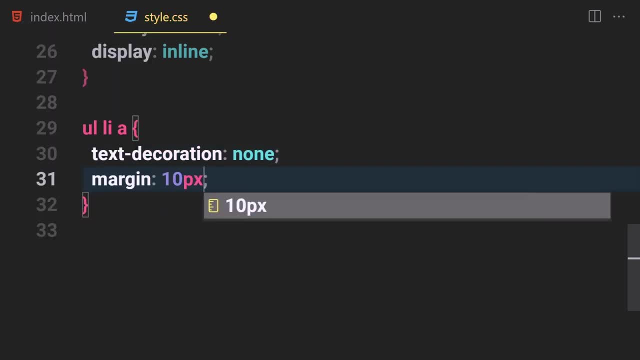 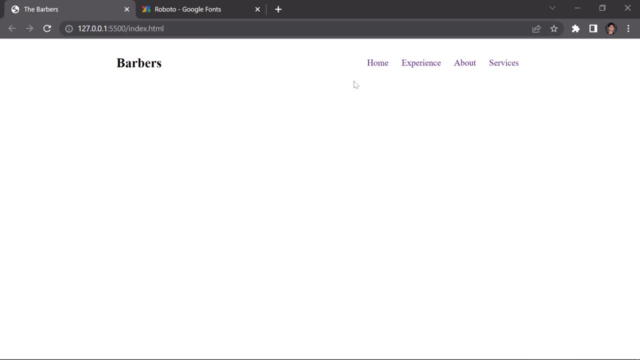 a margin for all of that. so i don't know, like maybe 10 pixels module will be fine. so if you save that, yep, 10 pixel margin is okay. so let's just see what else do we have to do? i'm going to change the color to totally black. so i'm going to write like: totally black color, yep. 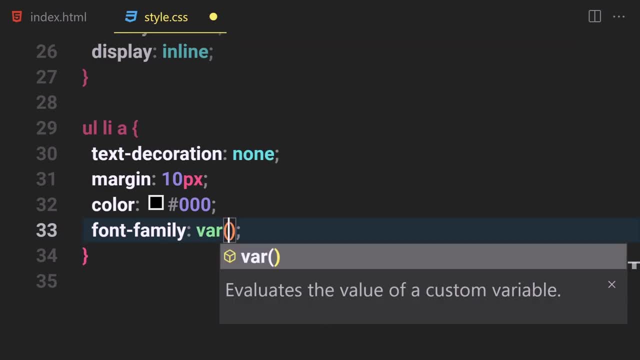 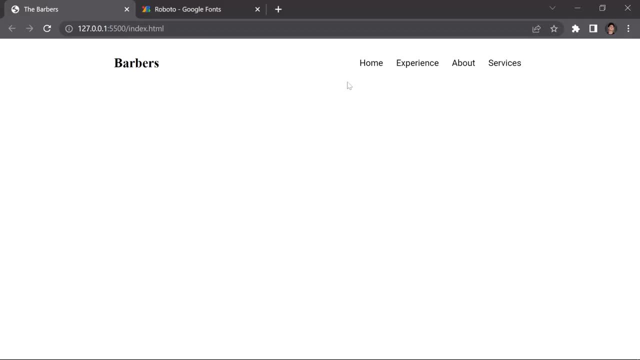 and also the fonts family is totally ugly, so i'm going to use that uh secondary font in this case. so if you save that, yeah, everything is looking totally okay-ish. so we are totally done with this um navigation bar in here and you know, we can also increase this margin if you want to. 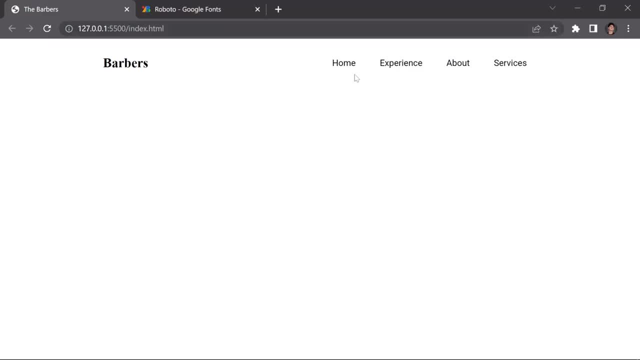 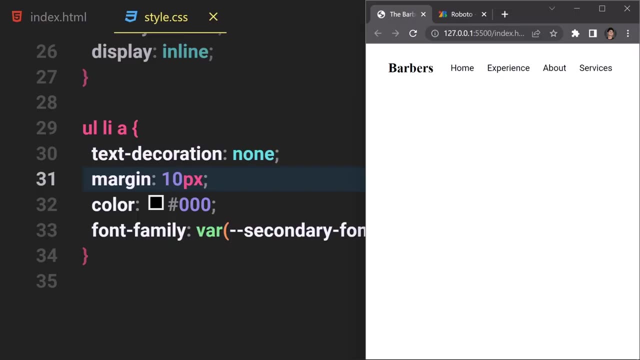 so let's just increase that real quick, save it. that's looking okay. but if you want to decrease this, so that's on you if you want to. okay, this is looking ugly. let's just write 10 pixel now. this is looking better anyways. so i guess that 10 pixel will be fine, if you want to increase or. 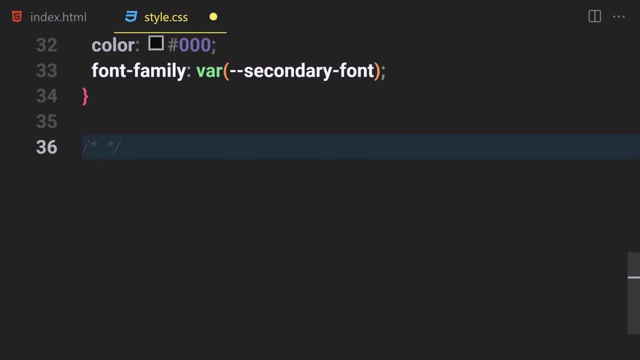 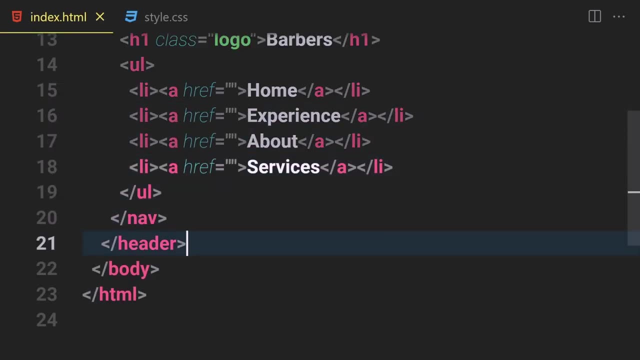 decrease that. so feel free to do that by yourself. and now let's just write a comment for yourself like navigation, and. and now let's just start working on our first um, what do we call it header area? so we already work with the header area, so now let's just start working on our first. 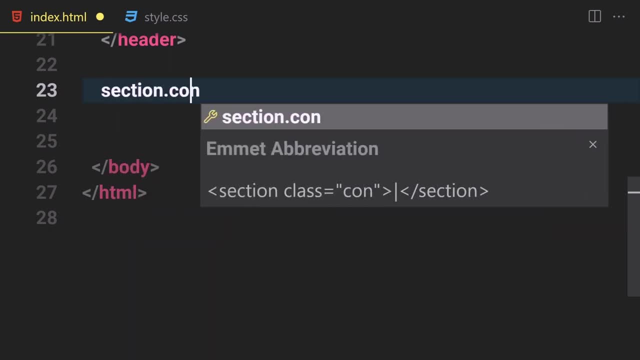 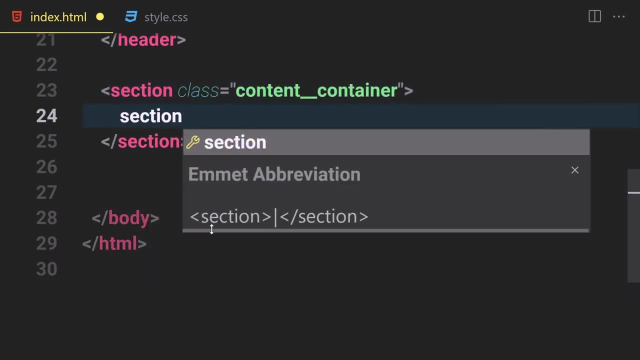 section, to be precise. so we are going to be using a section with a class of content and then dash dash and then container. okay, so inside that we are going to be using a new, new section, so we are going to be given a class of, like header and dash dash content. oh, my goodness. 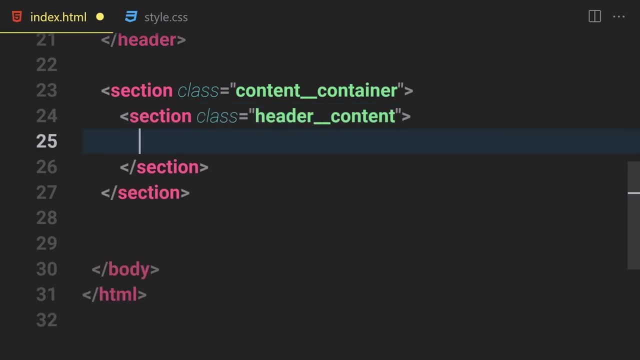 c o n t e n t, like that. now, inside there, we are going to be using our header and then heading, okay. so inside there, we are going to be using, like the, and then br for breaking, and now let's just use bar birds, okay. so, if you know what, we're not going to be saving that right away, because that's. 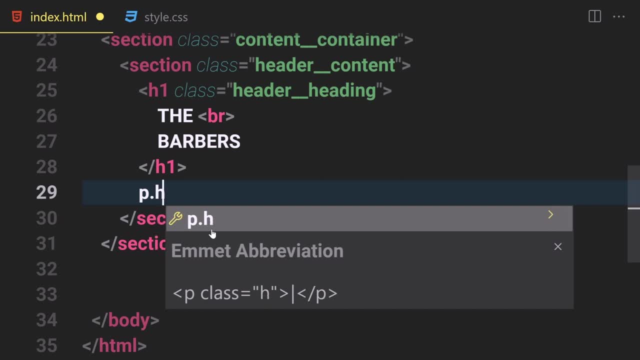 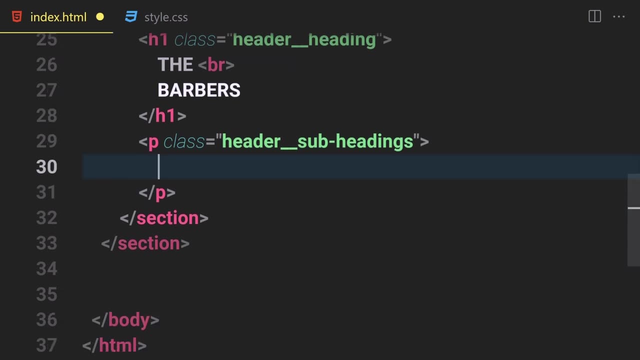 going to be looking awful. let's just write our paragraph in here and we have to give him a class of header sub and head dings. okay, so now let's just use like: uh, i'm gonna, you know, i'm gonna- fill it out and then i'll just see you in a second. okay, and what, chef, men's and boys, 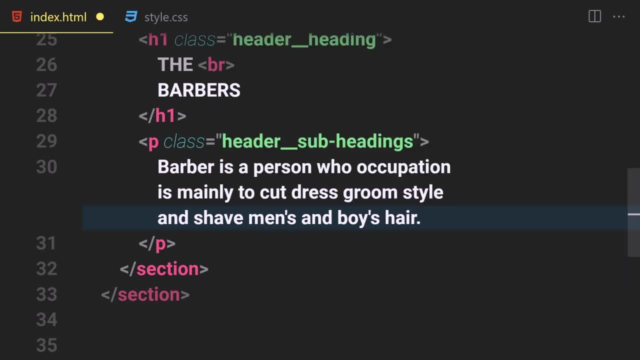 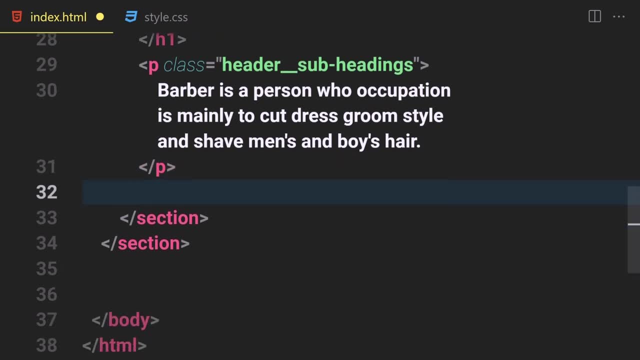 hair. and, by the way, this definition came from, uh, i guess that came from, uh, google. i'm not sure about that, but i just get there, i guess from a google you. so let's just write a container for buttons. so we are going to be using button container. 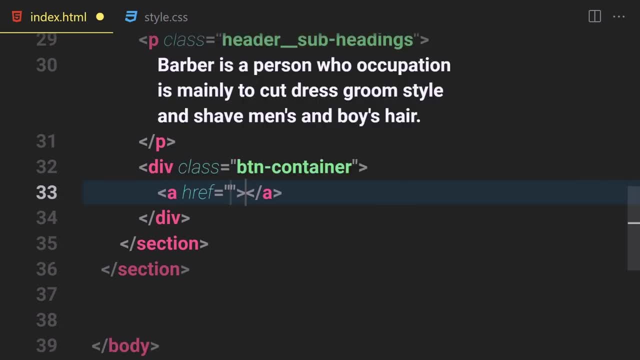 and inside that button container we are going to be just placing our one button with a class of main btn and it will not go to anywhere. so now we are going to have to give some sort of a label like i'll learn more. and now, if you just go back, and this is how our html coding looks like. so i'm 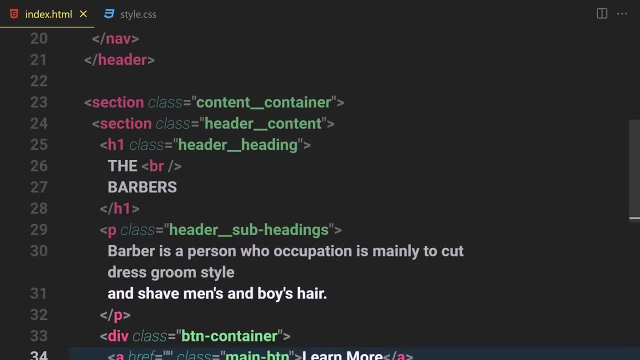 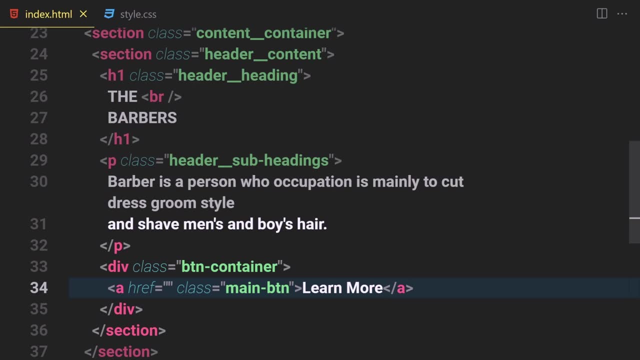 going to save my file and this is how it looks like. first of all, we have a section with a class of content- container. then we have a section header container and header content to be resized. then we have a header headings. then we have a header uh- subheadings. after that we have a 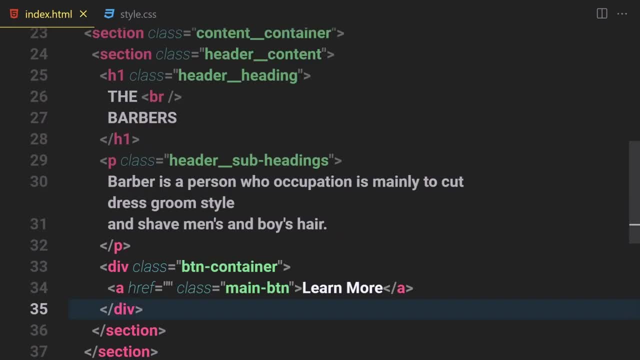 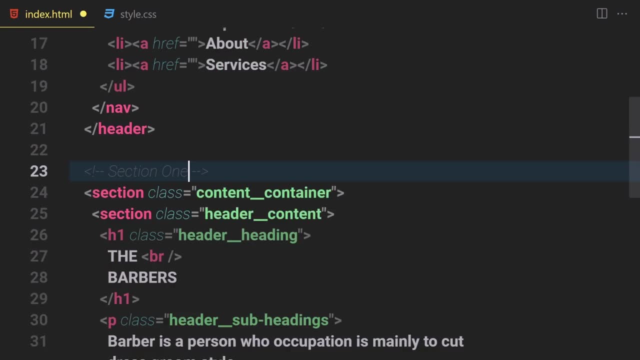 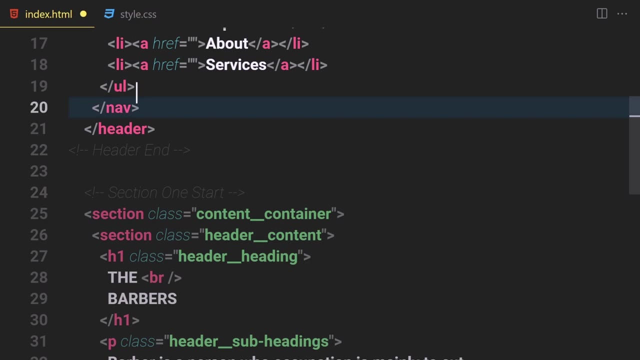 buttons container. we just have a new class of main btn. so now let's just get into our css, or you know what? first of all, let's just write: or section one, uh, start would be fine, section one start, and this is going to be header. and and also let's just use nav and uh-huh. you know what i'm going to. 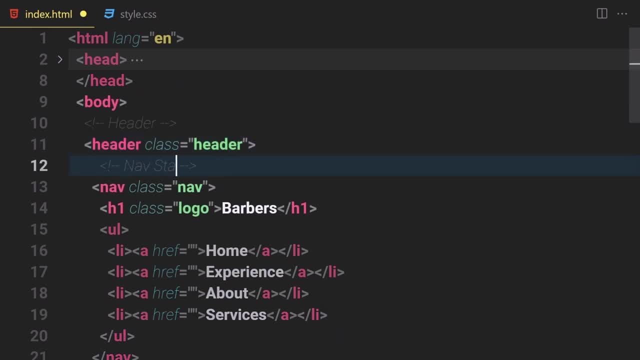 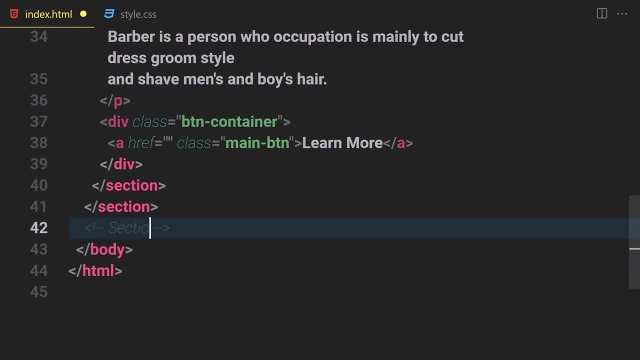 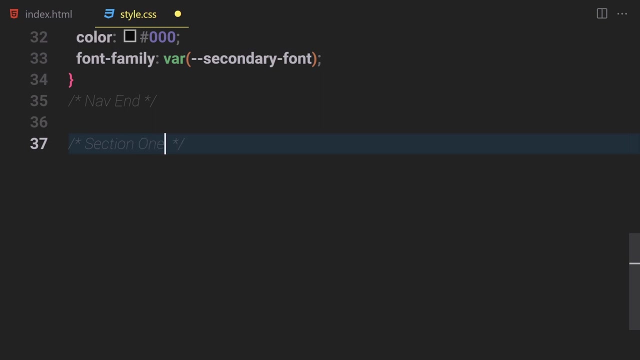 also put a comment in here just for you guys: nav start and nav end. underneath this section i'm going to also put like uh, section one, end, and let's just go to our css, write a section, uh one start and also let's just duplicate this line of code and this is going to 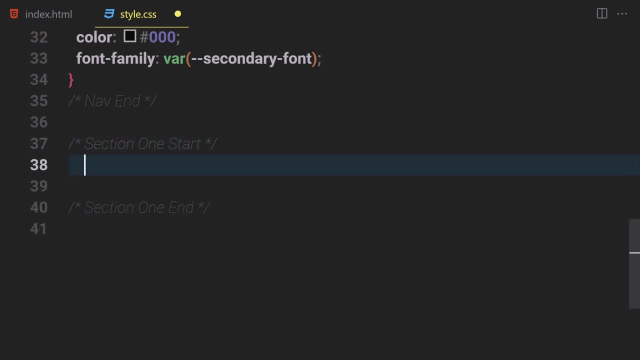 be section one end. all right. so now, inside this section, we are going to be writing our code. so what do we have to do first of all? first of all, let's just select our content and then container c-o-n-t-a-i-n-e-r. like: so this is going to be that container. let's just see. 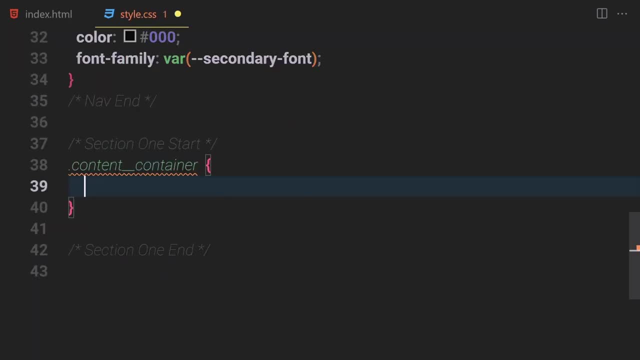 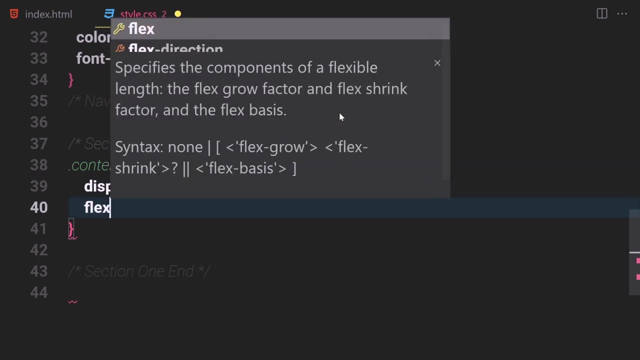 this content container and i'm making sure that i copy the exact same style- or class to be precise, not style- and now let's just use a display of totally flex, and flex wrap will be now set to wrap, because we want our items to wrap. so we are going to be using justify content of center. 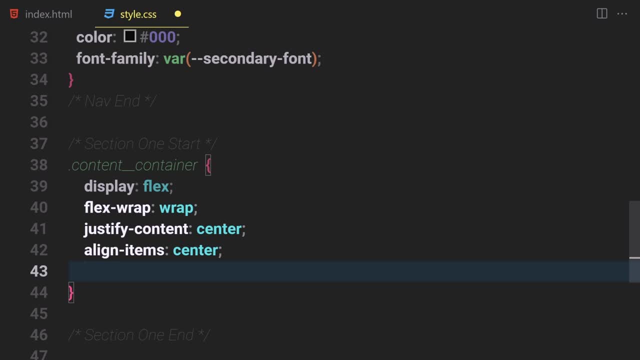 and also align items of center, because we want everything to be perfectly at the center. and now let's just go to our css. and let's just go to our css and let's just go to our css and let's give a little bit of height, like, i don't know, maybe 80 viewport height would be fine. so if you, 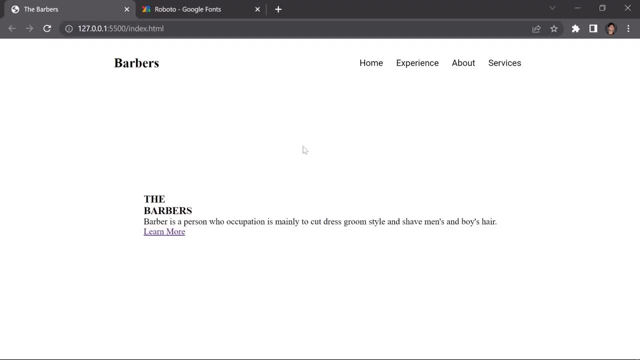 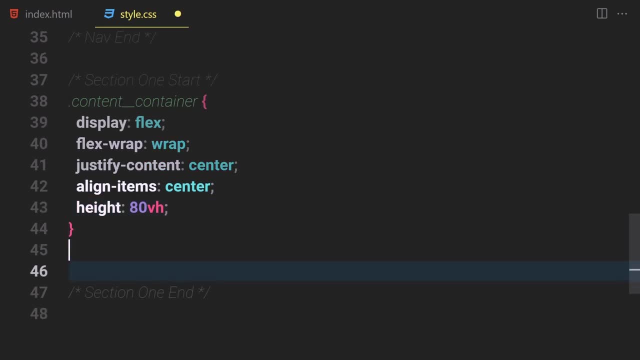 save that and this is how currently things looks like. all right, so now let's just get into this header content. so i'm going to just copy that from here, and what do i have to do? i'm going to just write dot or period or whatever you want to call it, and now let's just use a display of flex in. 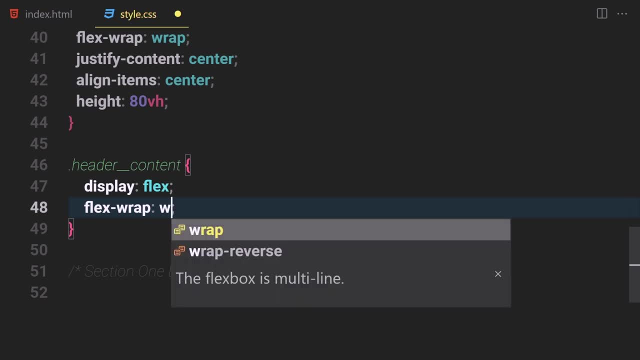 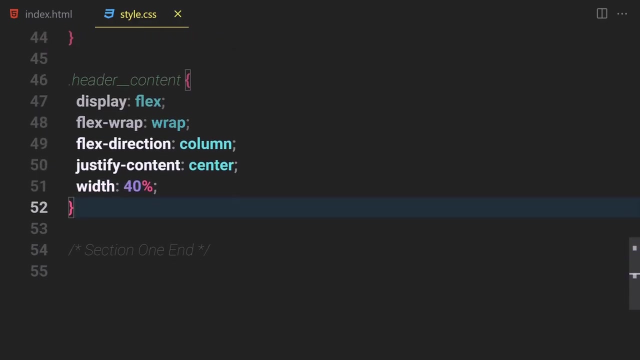 here. flex wrap will be wrapped, flex uh wrap will be wrapped, as i said, and flex direction will be to columns and justify, and i'm going to give him a width of like- uh, i don't know- 40 percent would be fine. so if you save that- and this is how it looks like- i know it's ugly, but guess what we are going to be styling- 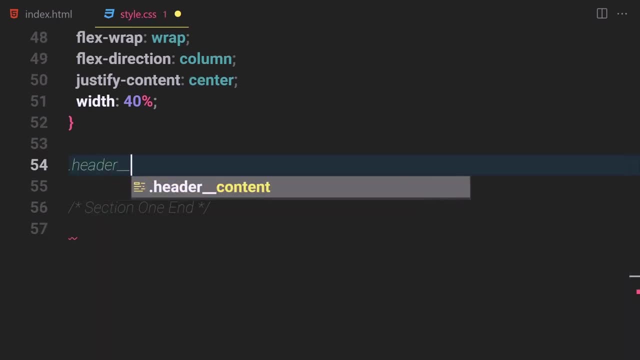 there a bit more. so now let's just get our header, and what header heading? which is this class, by the way. so we are going to be now styling this class, all right. so what do we have to do in this class? so we have to give him a width of like 70 percent, and now let's just use our font family. 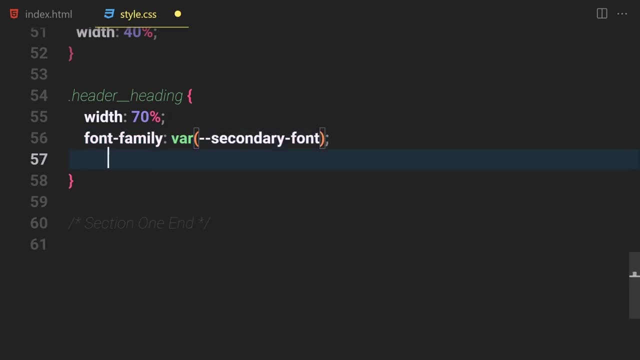 and give him that. uh, what do we call it? a secondary font family. there we go and we are going to be using a color of rgb or which is 82- uh, yeah, 82, i guess. so not 81. so 82, 82 and 82, all right, so i'm. 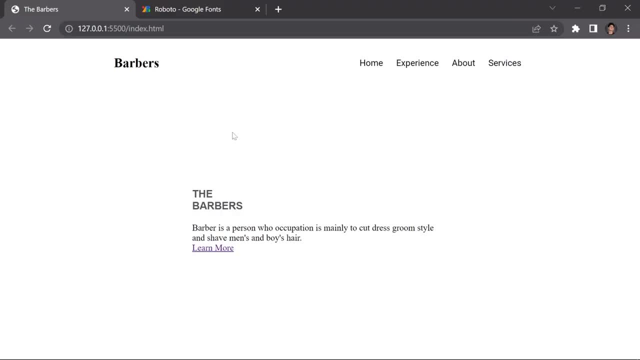 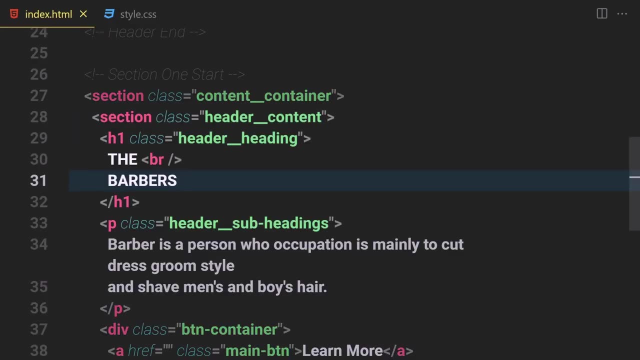 going to give him a margin of 20 pixel for top and bottom and for left and right. we would have word zero, all right. so this is how it looks like and we selected that as a header heading. uh, but i'm not sure whether the all right. so this is a header headings and this one is a header head subheadings. 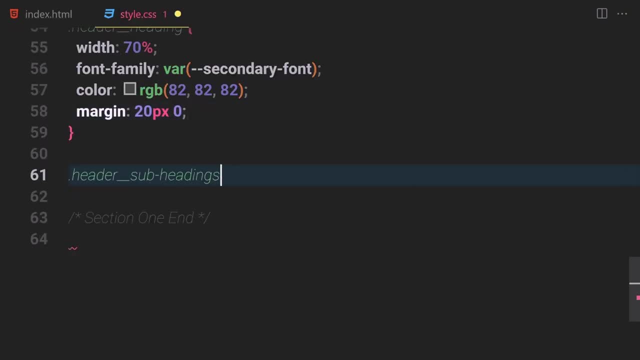 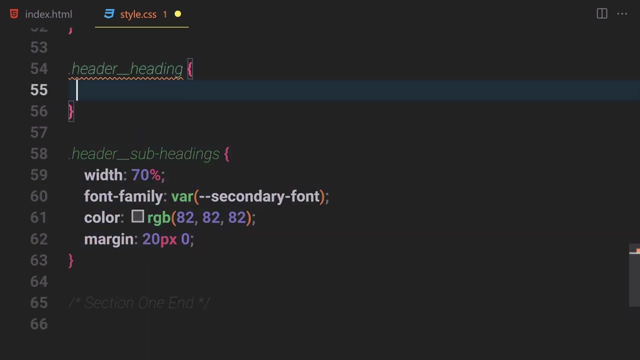 so i'm going to copy that one for now, and now, let's just select that. and what do we have to do? we have to give him a width of that one. you know, i messed it up. i messed it up this styling. i'm going to copy or cut all of that styling and this styling will go up here. and what else do we have? 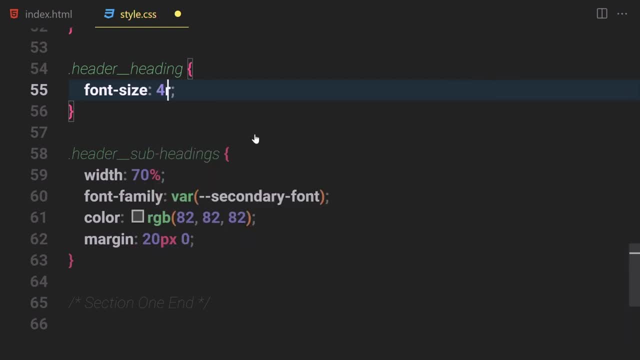 to do? we have to just increase the font size and we are going to add some more lines andать to this font size to just like 4m. and font family: this is going to be the font family of war, of main font, so we are going to be using our main font in this case. so if you save that and this one is, 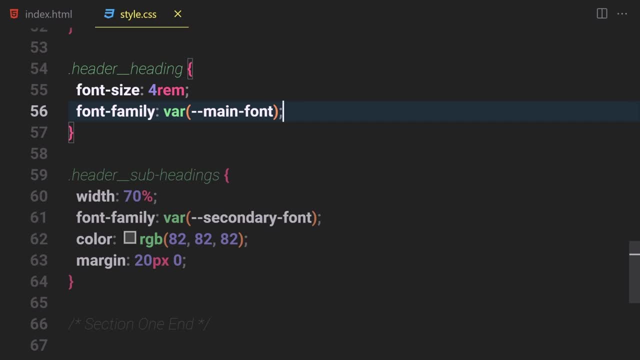 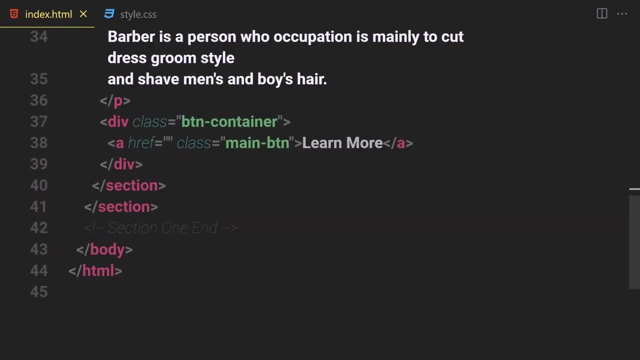 looking massive and the other one is looking totally cool. and now let's just work on our header image. so you know what? for that we have to write a little bit more coding inside our html. so we are going to be writing not outside from the last section, but inside the last section, i mean. 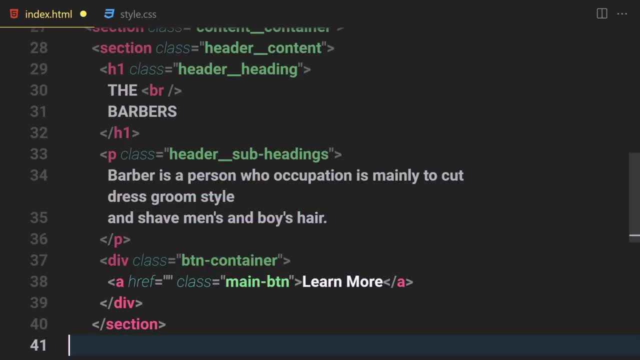 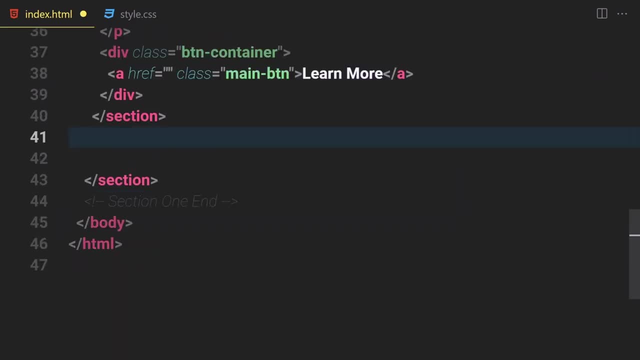 like inside this section, but outside from that other section which is called, like a header- not a header but a header content section. so and so, outside from this header content section, we are going to be creating a new section called header image. so we are going to be placing our image in 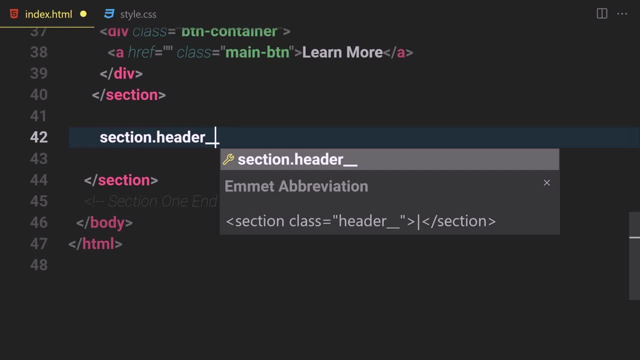 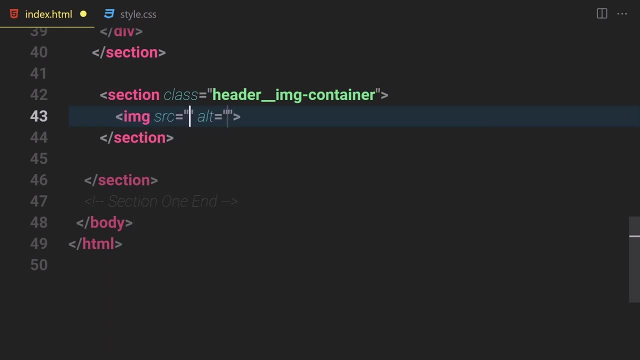 here. so i'm going to just create a section with the class of header and then dash, dash, img and then container. so we are going to be selecting there, but before we do we have to render our image in here. so i'm going to just hold ctrl and hit space and i'm going to go to my image. 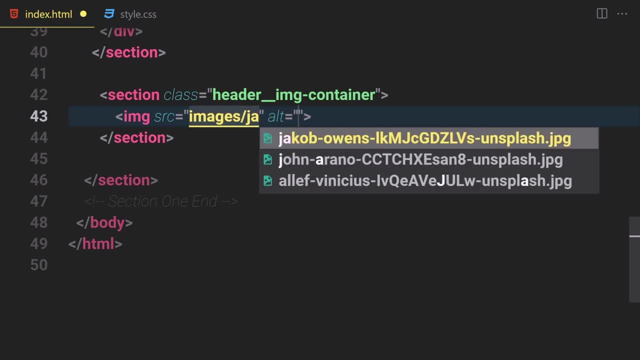 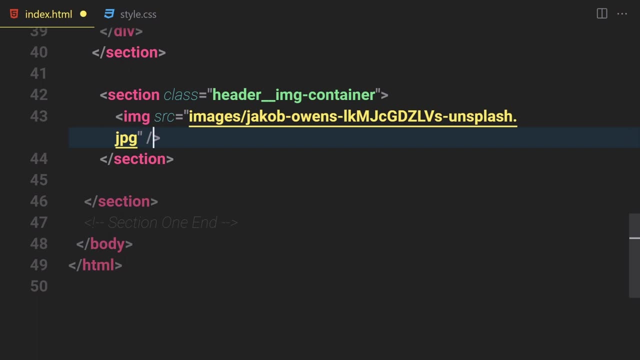 images folder. and now let's just select that jacob uh person. so i'm going to select this image- and, by the way, all of these images will be inside my java repository, if you want to check that out- and i'm going to also give him a class of what? class of header, and then dash, dash, img and also. 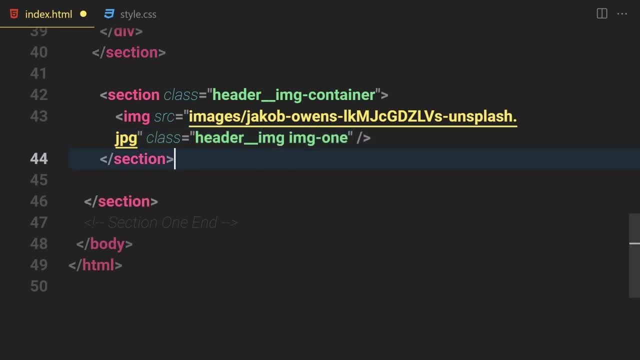 img1. okay, so this is going to be our image1. and now, uh, underneath this image, let's just create a new image. so i'm going to just write image. and now let's just hit control space, go to the images. and now let's just select that- stephen lewis or whatever the guy name is. let me just write a class. 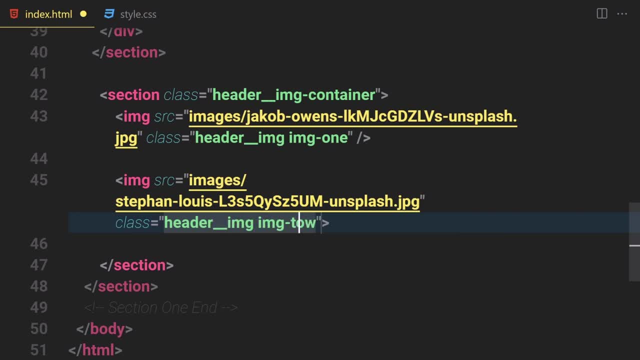 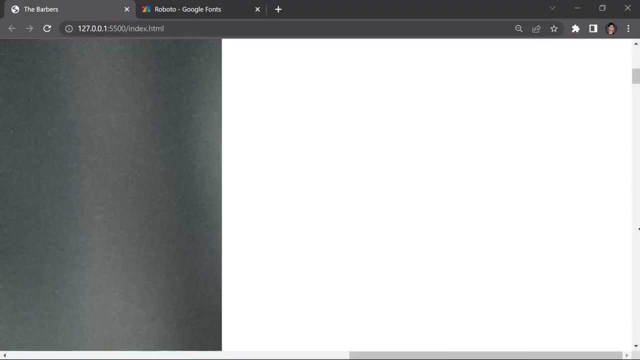 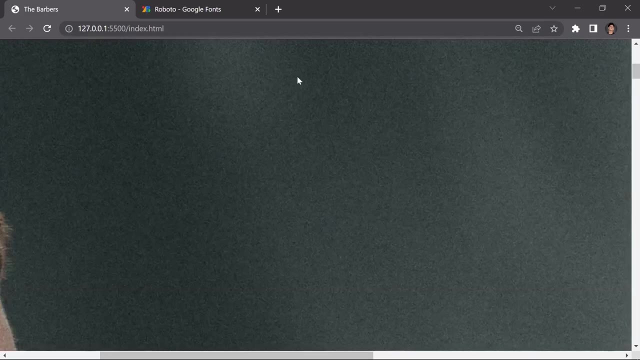 of header: dash dash image and also img2. okay, so 2, and now let's just start working on that. so before we do look at these images- these images are supremely long, so supremely high quality images- look at this guy. so now let's just start working on our css and then you will get to know. 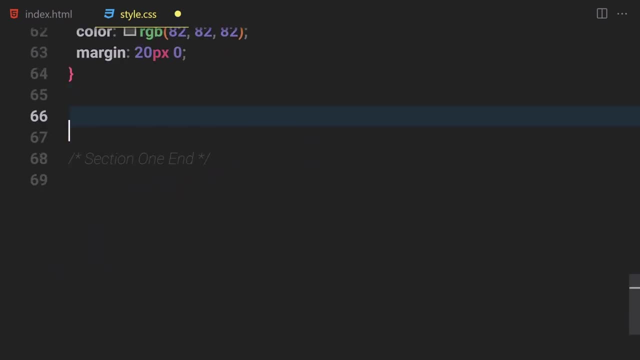 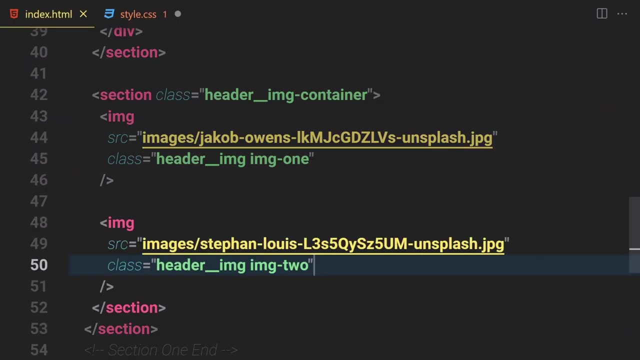 what can we do with that? so now let's just start working on our css and then you will get to know work on this section. so first of all we have to select that header and then dash, dash img. so which is, uh, this header img, where are you header img? so we have header img right here and we have header. 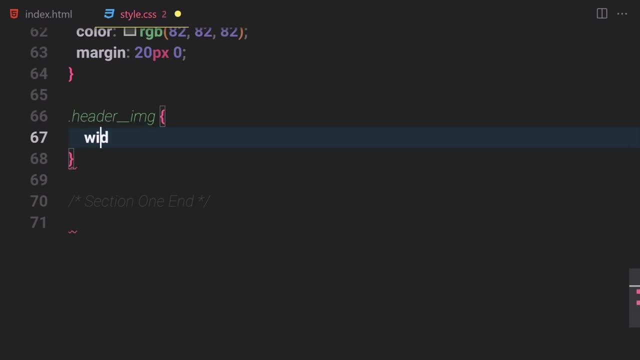 img class right here now. let's just select that. give him a width of like 200 pixel and height. in this case, i'm going to give him a height of like uh, 300 pixel, maybe. so, if you save that and let's just wait for it. so this is how currently images looks like. all right, so now. 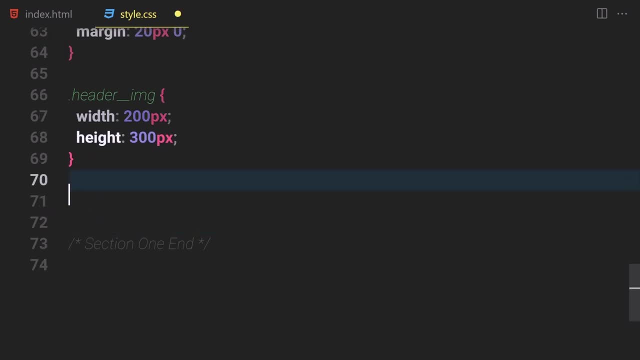 let's just select our header image container first of all. or you know what? we are going to be selecting the above, because this is the main header uh container. so let's just select that and i'm going to paste it right here. so we have header image uh containers. so i'm going to give 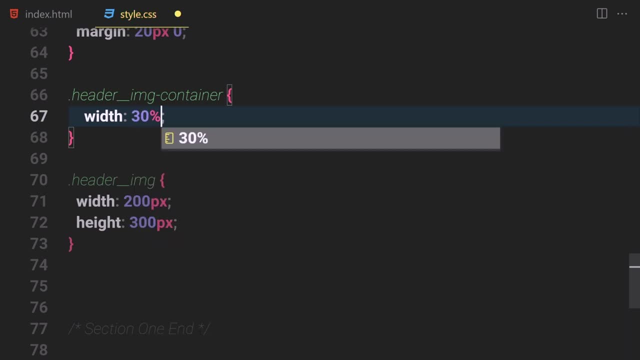 a width of like maybe 30. let me just write 30 in here, and i'm going to also give him a height of like 50 vh, and the position in this case will be relative. okay, so now? what else do we have to do now? let's just select our 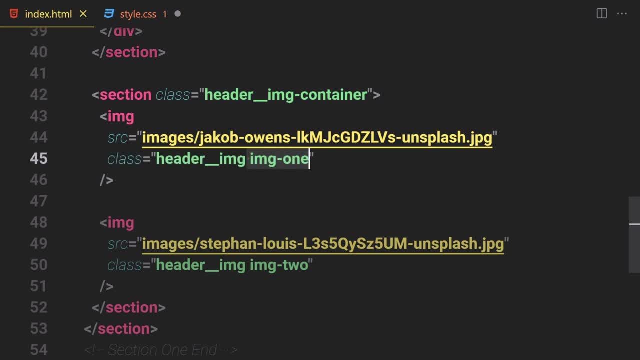 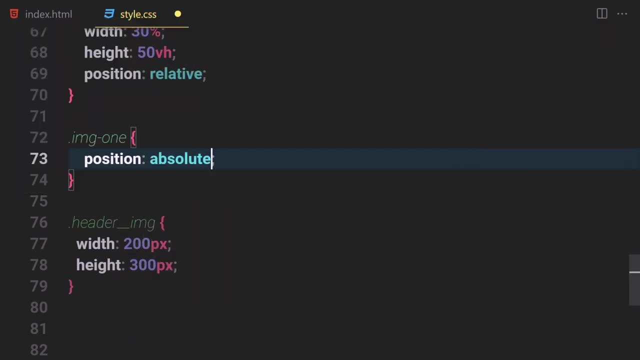 image one, so img one, which is this class right here. okay, so now we selected that image. what do we have to do with that? so we are going to be using a position of absolute in this case, and now let's just write a left to ten room. okay, so this is going to be the first image. so if you save 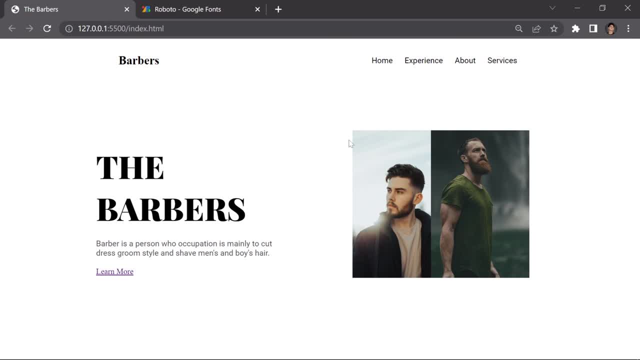 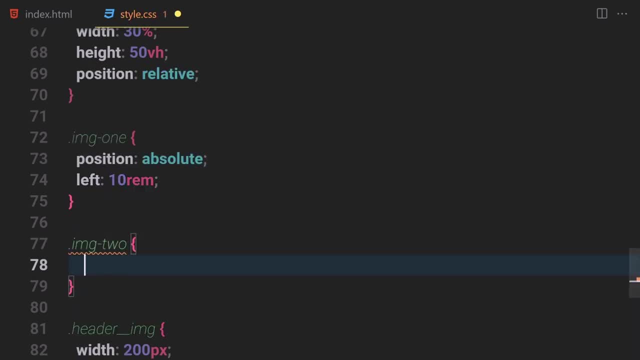 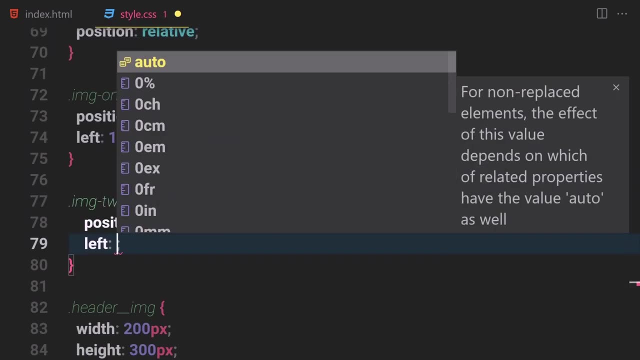 that and this is how it looks like right now. okay, so now let's just work on that second image, which is that img, two clones. so let's just select that img and then select or two, and let's just use a position of what position of absolute in this case, and right of left to 30, not 30 room, but just at. 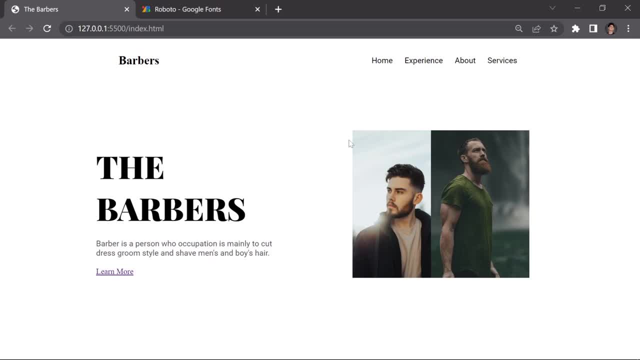 3 ram and top value will be just at ram. so if you save a file and boom, this is how it looks like. but if you just give a little bit of uh margin, not margin, but a height of like 100 vh, so it will look cool. you know what? you will see that in a second. so now let's just style this. 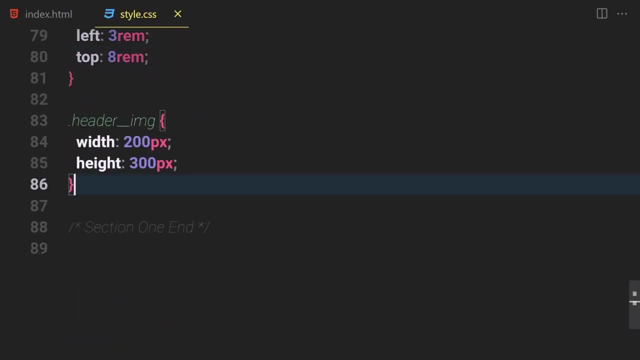 uh button real quick. so we are going to be selecting that button first of all, which is that main button. begin a class of main btn. i'm going to copy there and i'm going to select that right here. so what do we have to do with this? we are going to be using 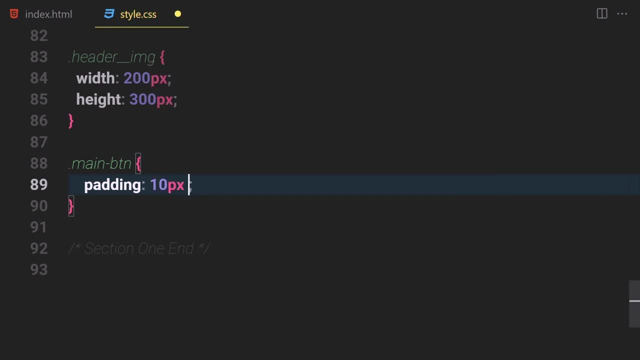 not a padding in line, but padding. so padding: 10 pixel for top and bottom, 20 pixel for left and right, and text decoration. we want to remove the ugly border, the background color we are going to be using, or on- oh my goodness, bg, god damn. so war will be now main color and let's just remove that. 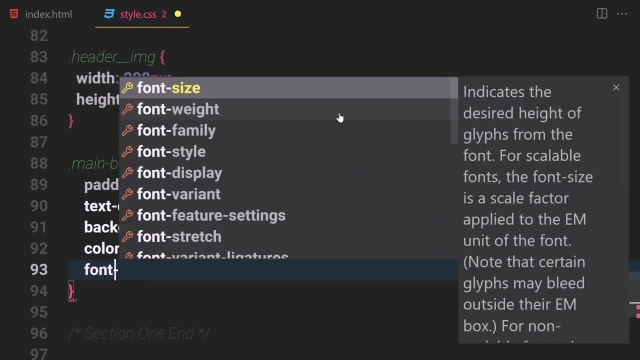 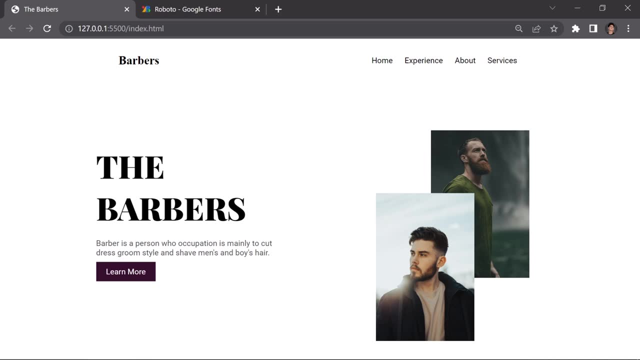 and color will be now, in this case, totally white. i'm going to use a font- family of war- and totally secondary fonts, if we save that, and this is how it looks like right here. i know we can provide crazy styling in here, but for now this is totally looking better anyway, so i guess we are. 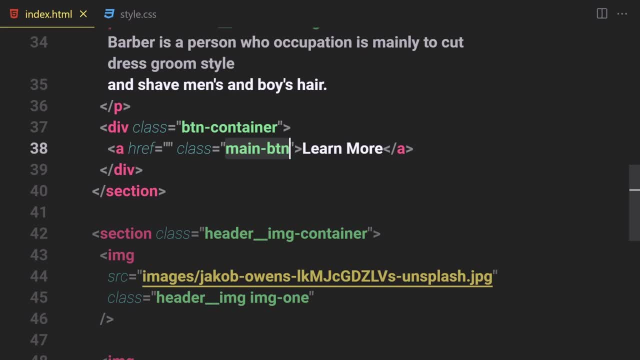 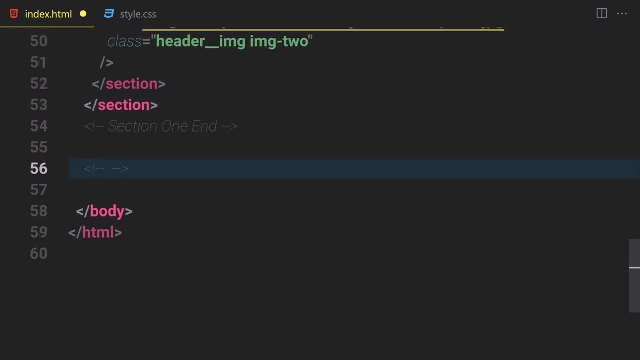 totally done with this header section, and now let's just get into the experience section real quick, all right. so outside from this uh, section one, i'm going to create a new comment for myself which will be like a experience: experience section start. and now let's just write, first of all, a 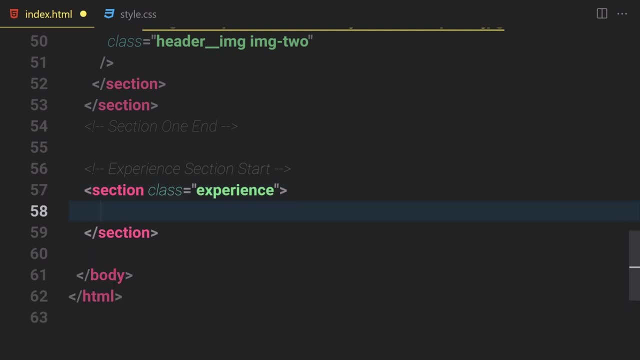 section, with the header section, and then we are going to start with the header section, and now we are going to start with the header section and we are going to start with the header section. a class of experience. And now inside there we are going to be creating a new class, not 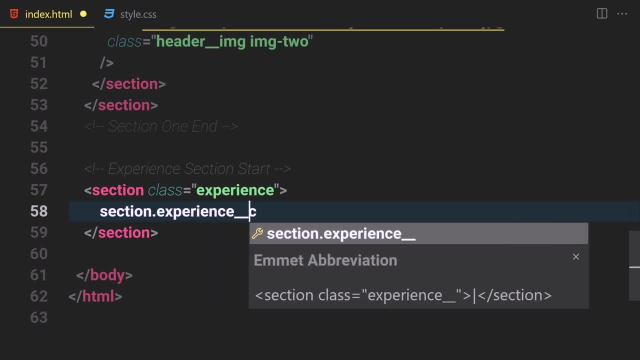 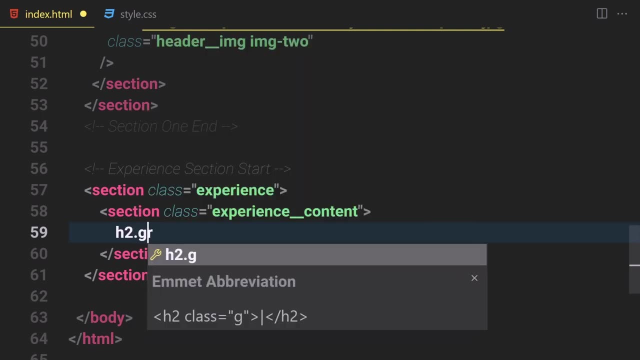 a class by the section, with a class of experience and dash dash content. So inside this experience content, we are going to be using h2 in this case and which will be like I don't know, gray and heading. So let's just give him a value of 30 years, 30 years. And now let's 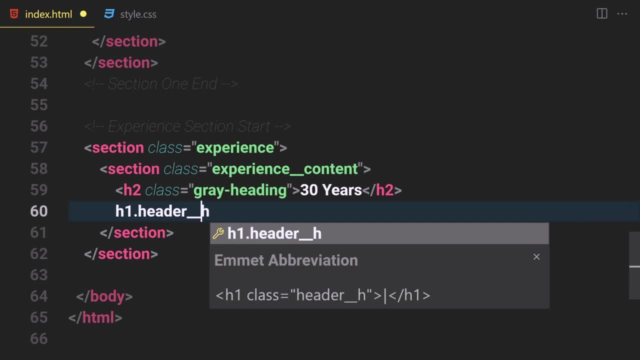 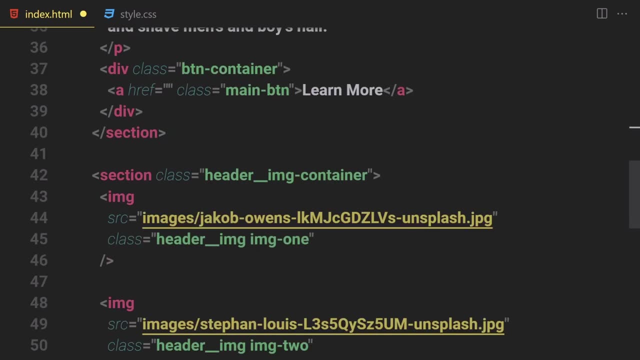 just use our h1 with a class of header and dash, dash heading. So we are going to be using this class, which we style right here, So we have that header heading class right here. So we are now reusing all of their styling right here, So we have a heading not hitting. 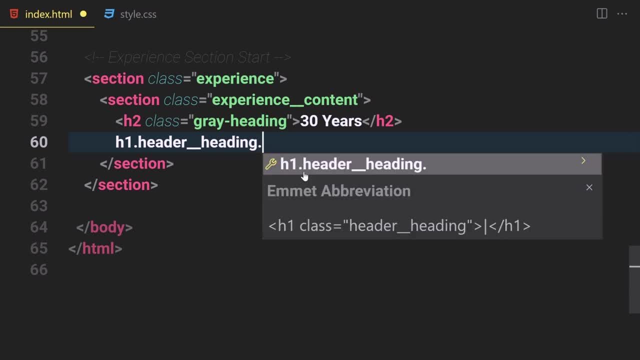 Oh, my goodness, what the hell is wrong with header heading. So now let's just give him another class of experience heading, So x periods, and then not dash dash, but just a single dash would do so experience heading. Now, inside this class we are going to be 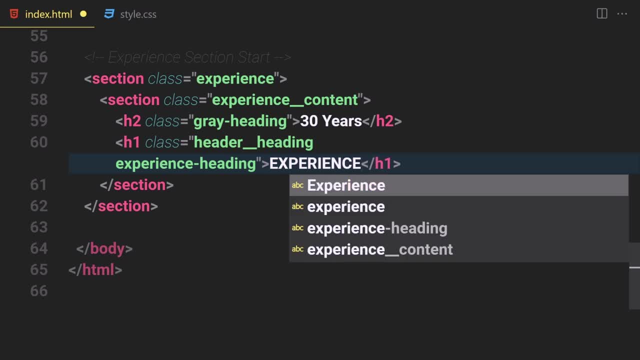 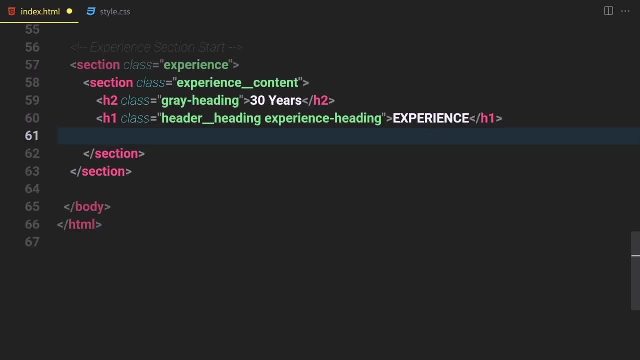 just using experience in uppercase Underneath this h1.. You know, I'm going to just zoom out a bit so you guys can see everything a bit better. And now let's just use a paragraph with a class of lowercase paragraph with a class. 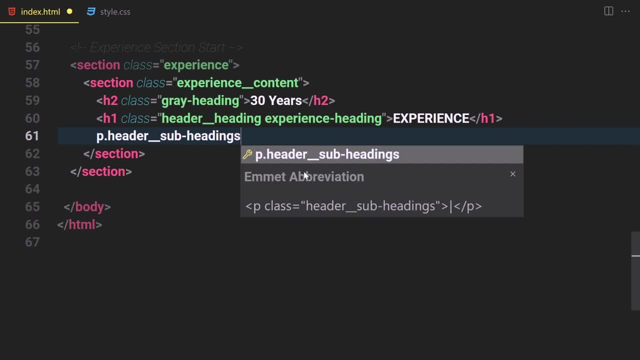 of header and then sub headings. we are reusing that class which we selected above, and then experience, experience, exp, E, R, IE and C. there we go And then experience subheading or s to be precise. So headings plural, plural, whatever. So barber is a. 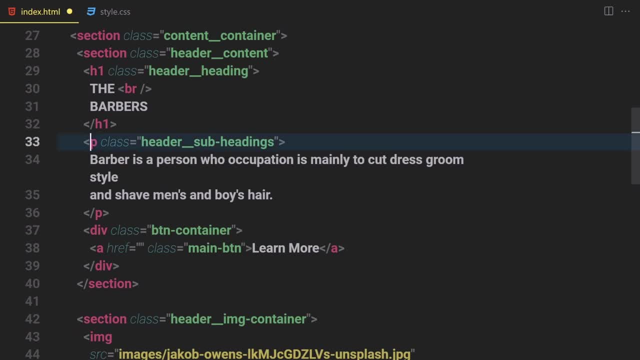 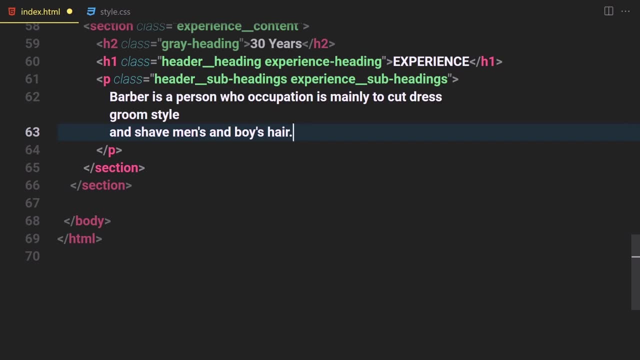 person who you know. I'm going to copy that. I don't have to rewrite it again and again. I'm going to copy there real quick and I'm going to pass it right here. Yep, that's cool. Now, underneath this paragraph, what do we have to do? we have to write a section with: 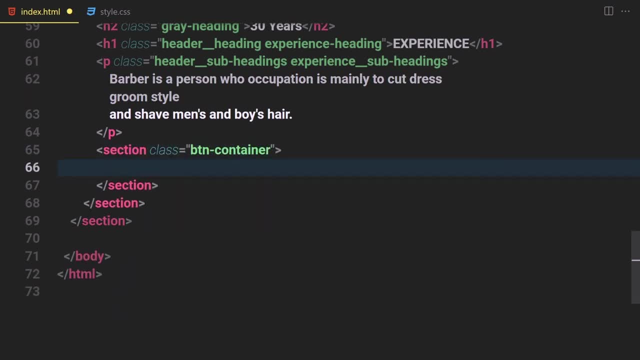 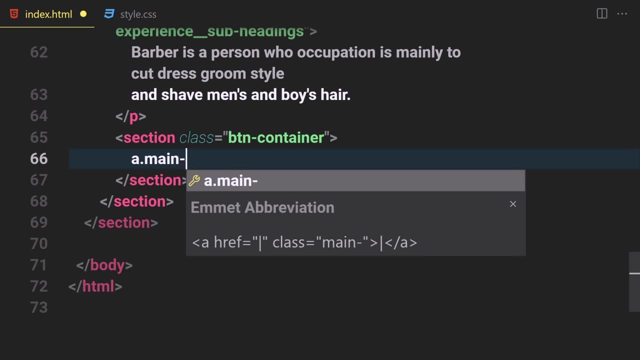 a class of BTN container. So we are going to be reusing the BTN container class which we use above. So now let's just create an anchor class, I mean like anchor, with a class of main BTN, And we are reusing that button right here one more time. So learn And then 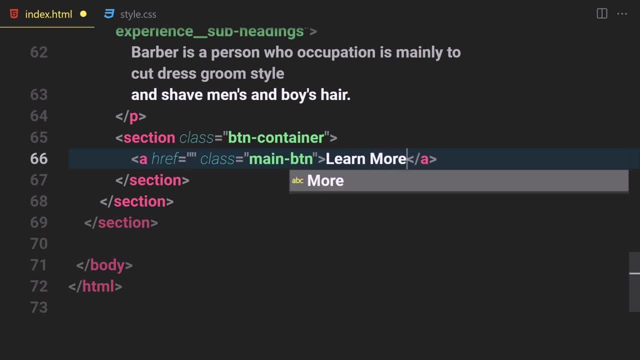 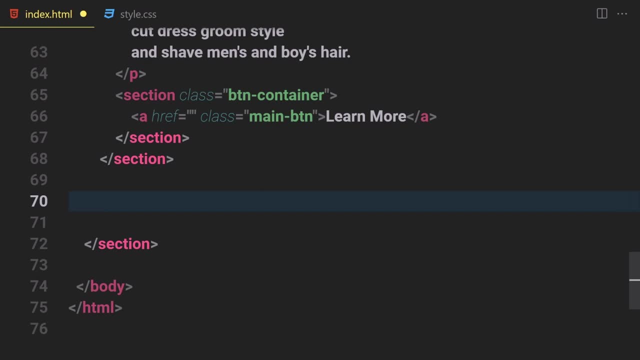 learn more, in this case, LEARN. Yep, that's fine. Underneath this section, or, you know, underneath this section, like all of the above, all of the underneath. So we are going to be using David, the class of experience, IMG, exp, E, R, IE and C- Yep, that's cool, All right. 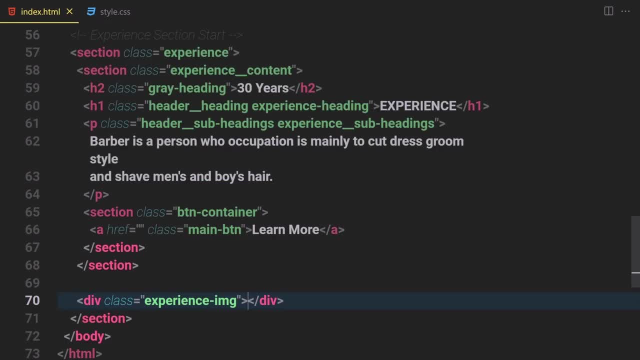 So now let me just show you everything, And then you'll get to know what I'm talking about. So first of all, we have an experience section right here, then we have an experience content section and we have a gray heading. So that's why I provide a class of gray heading And then we have. then we are reusing this. 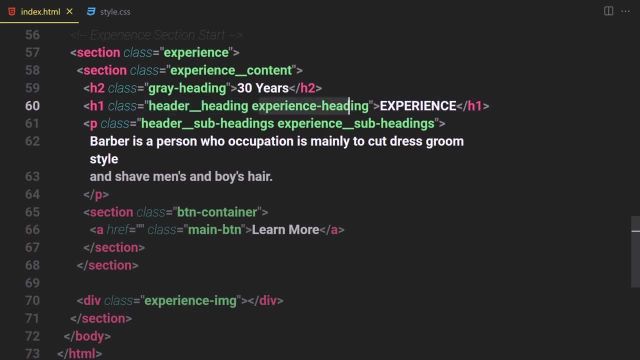 class from above, like header heading, And then we have a new class for this experience. then we have. then we are reusing this class one more time And then we have a new heading or new subheading class right here. then we have a buttons container. we are reusing this. 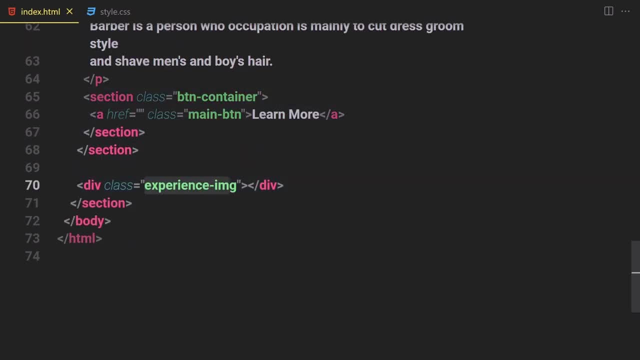 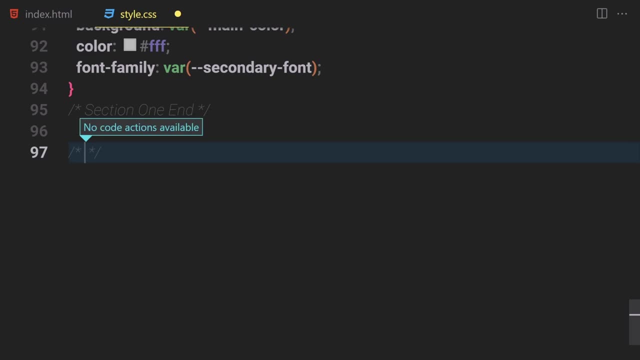 totally same clause, And then we have a new day with a class of experience image. Alright, so now let's just get into our CSS. And now let's just try that a bit. So I'm going to zoom in a bit. First of all, I'm gonna write a comment for myself, like, hey, I'm going 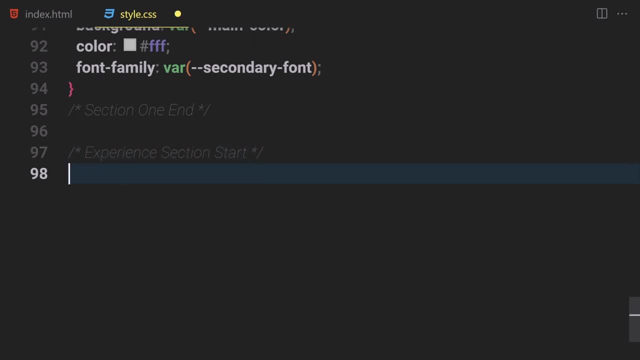 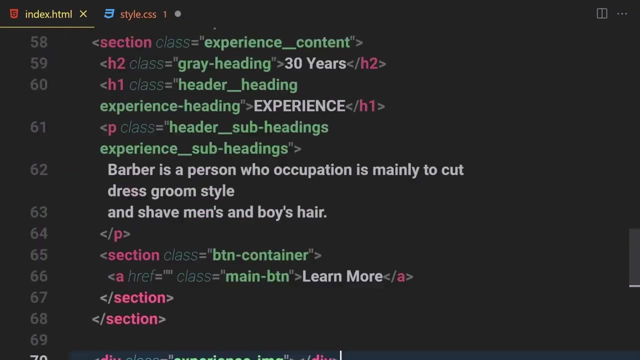 to say experience section start, And now let's just duplicate that and change it to experience section. in And inside this experience section, first of all we have to select or experience- oh my goodness- X, P, R I E N C- kind of a long spelling for this one. 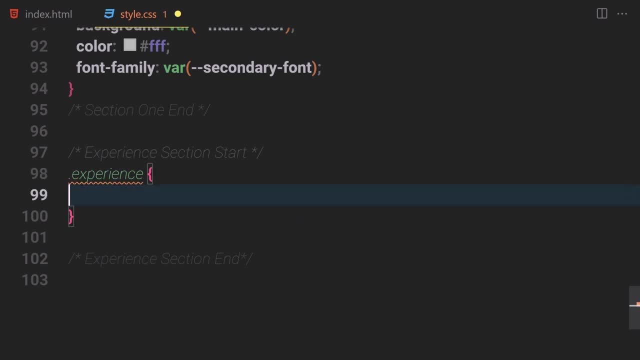 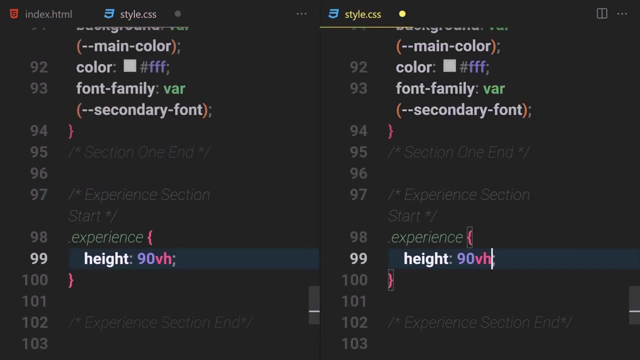 Let me just double check. So we have this class experience. Yep, both of them are fine. So, first of all, what do we have to do? I'm going to give him a height of like 90vh, like a viewport height. 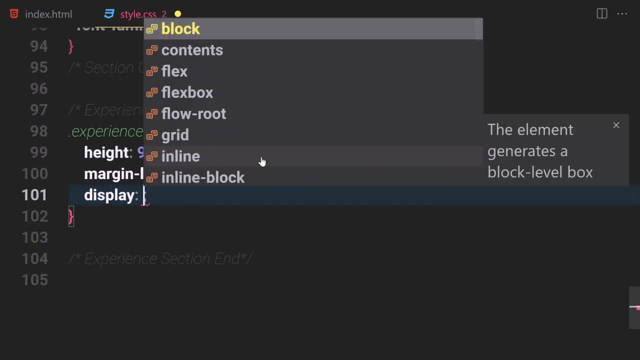 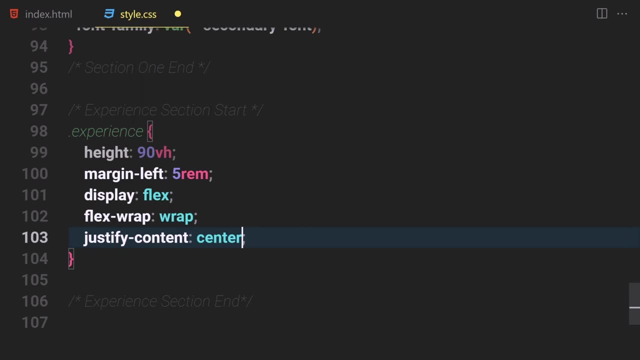 Now let's just give him a margin from a left, so like 5 frame would be fine. I'm going to give him a display of totally flex, because we want everything to be flexible. So flex wrap will be set to wrap, justify content will be now set to center and align items. 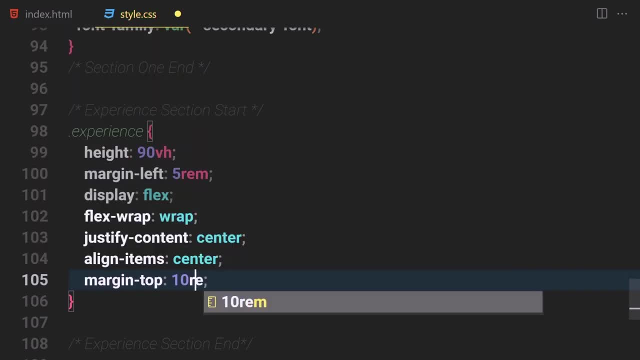 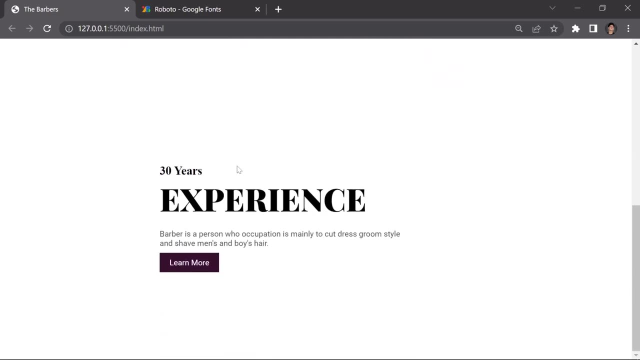 will also be set to center. So I'm going to just also provide a margin top of like 10 rim, because we want a lot of huge spacing in there. So if you save our file and it will take a little bit of time, and this is our experience section right here. So now 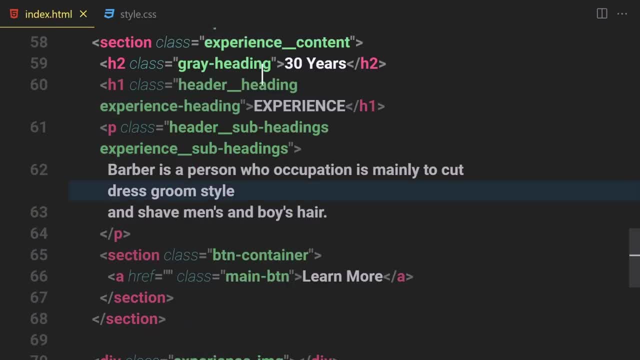 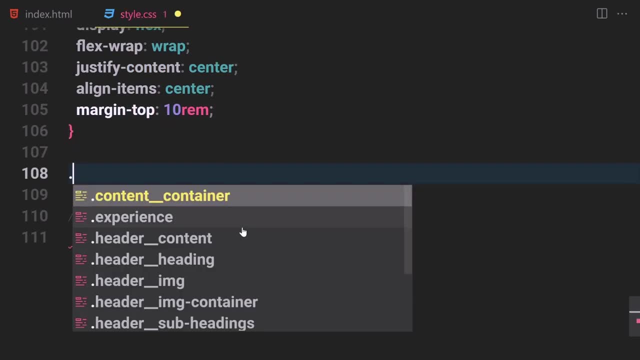 let's just style that experience image, which we provide right here, Experience IMG right here. So now let's just style that a bit. So we are going to be using exp. your regions are autocomplete is super awesome in Visual Story Coder And we are. 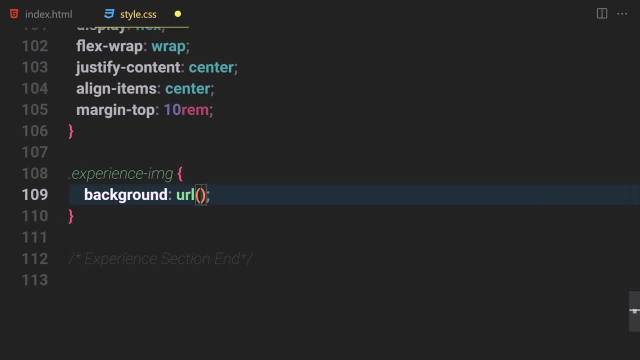 going to be not using a background color, but a background image of URL, And then let's just go into an images folder And we are going to be selecting that EU. Sorry, I can't pronounce your name, but I'm going to select this image And now let's just use the background. 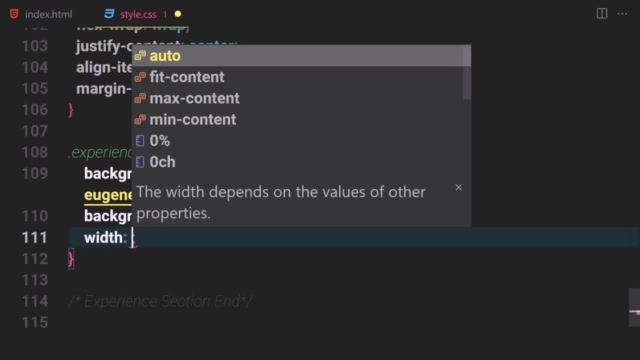 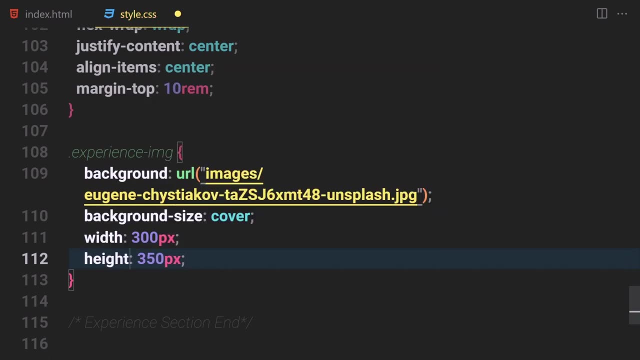 size of poorly covered And also provided with will be, like I don't know 300 pixel would do. and duplicate that and change this one to 350.. And this is going to be for our height. And now let's just provide a margin to the left, not to. 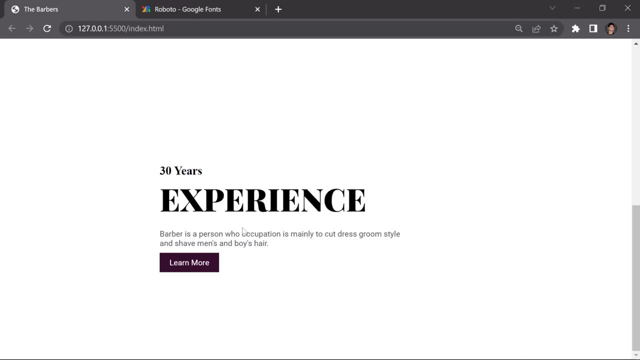 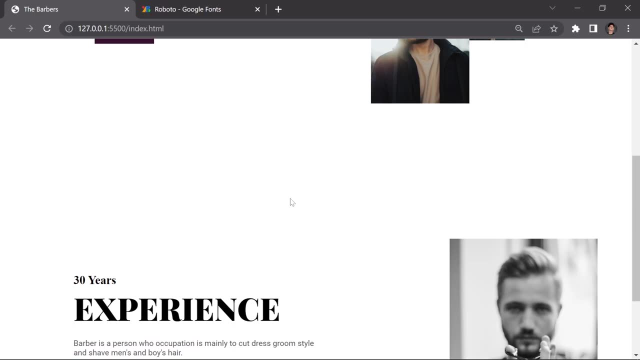 the top, but to the left of 50 pixels. So now, if you sell a file and let's just wait for it, So this is our guy right here And this is how his image looks like. Alright, so what do we have to do? So let's just style this gray heading. So we forgot that. let's. 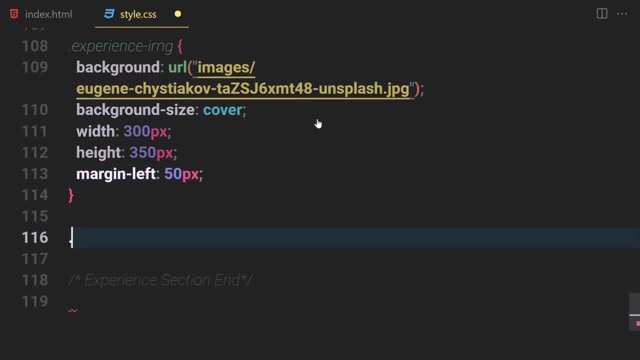 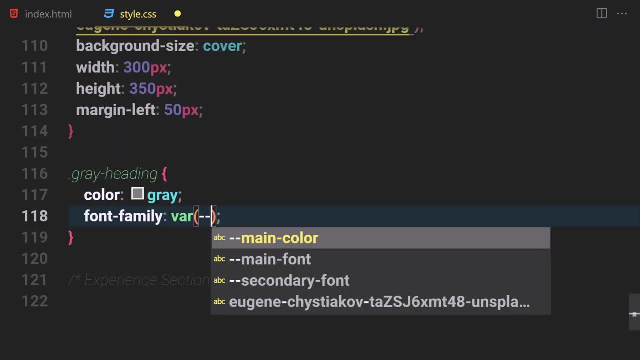 just copy it And I'm going to paste it right here, select it right here, to be precise, And let's just write a color of 40 gray And also the font family will be just a main font. So if you sell that and here you can see, this is how it looks like right now. Okay, 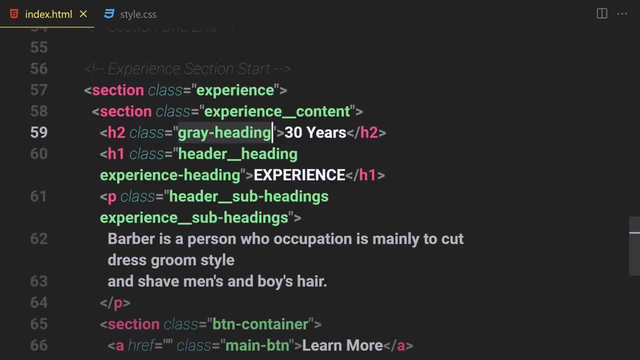 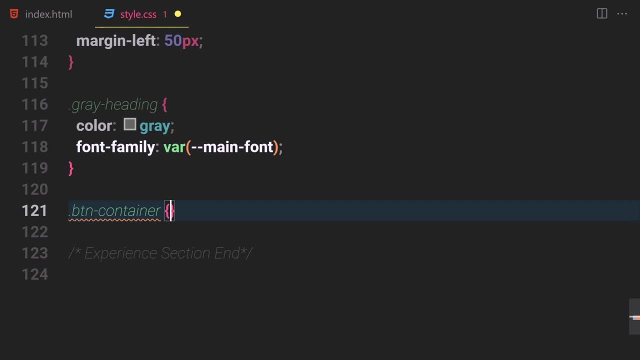 so what else do we have to do? we have to select the buttons container, which is this button container right here. In this case, I'm going to copy there And here. I want to select a real quick, And now let's just provide a margin for the top to be like: I don't know. 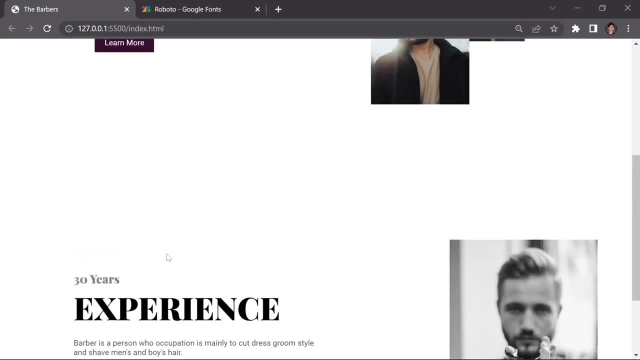 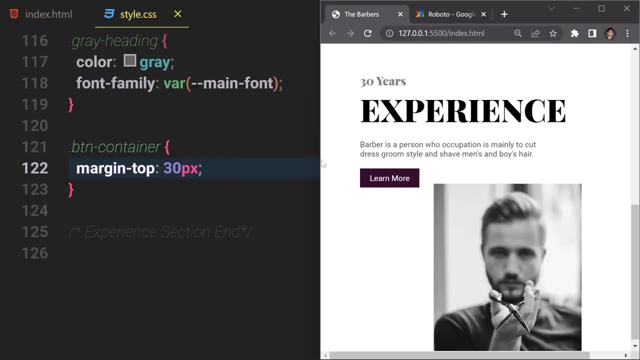 30 pixel would do, And if you save that, that's awesome. So now let's just copy that And then I'm going to paste it right here And this is how it looks like, And for now this will be not responsive if you check it. So this is not responsive. I mean like it is responsible. 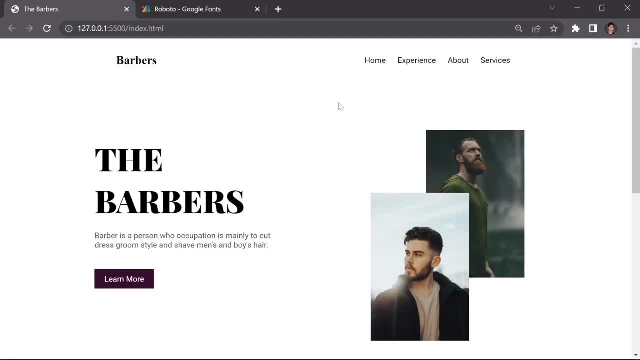 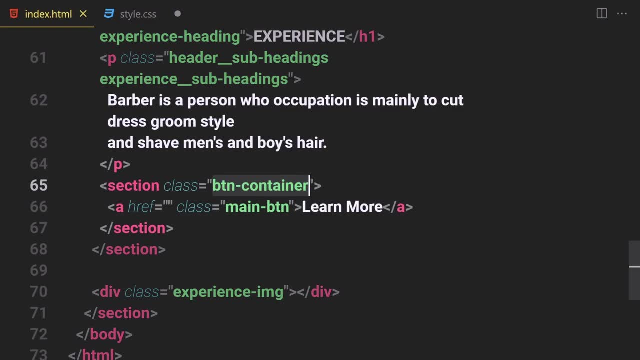 it's not looking that much great. So once we jump into a media queries, we are going to be making that responsive. So this is the end of our experience section. Alright, so now let's just get into a new section called what. So this is section is called a social. 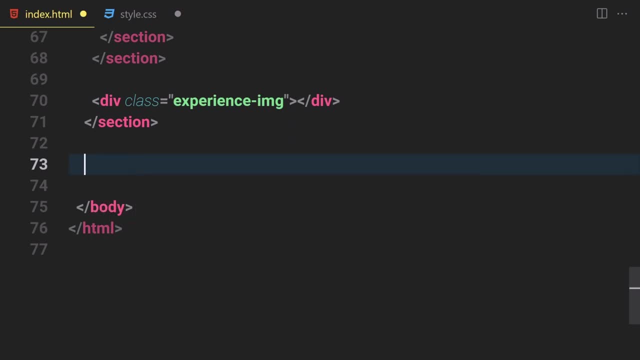 media or whatever you want to call it. So you're going to be creating a section, or you know what? first of all, you're going to be creating a section. you're going to be creating a section, So let's just write experience Section and R analysis, Right? 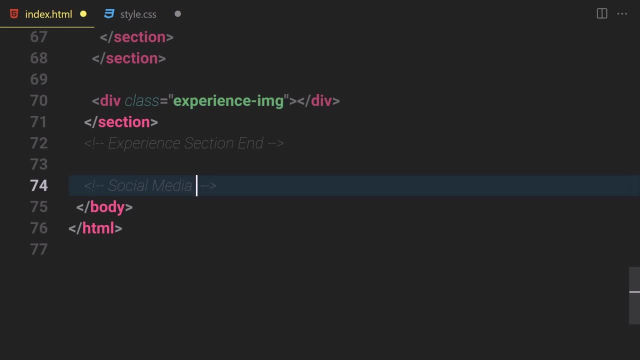 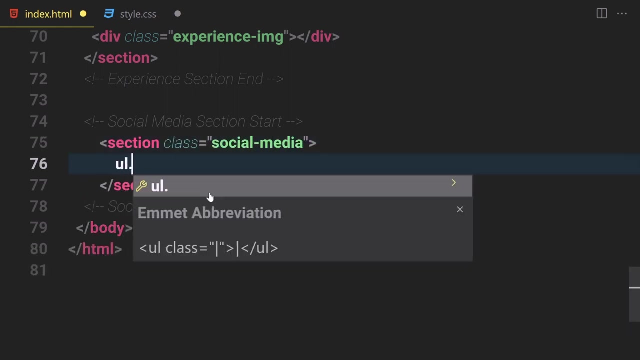 Social social media Section, start, duplicate that, And this is going to be the end of the social media section. I wish I. so let's just write a section with a class of social media Inside that we are going to be using ul, with a class of SM and container, And then let's 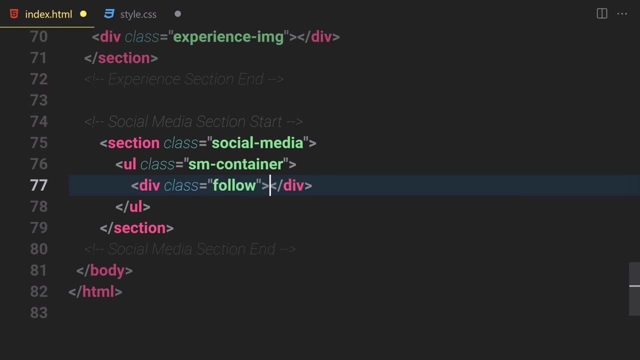 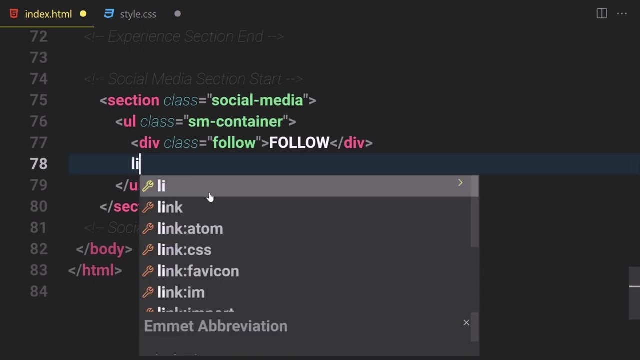 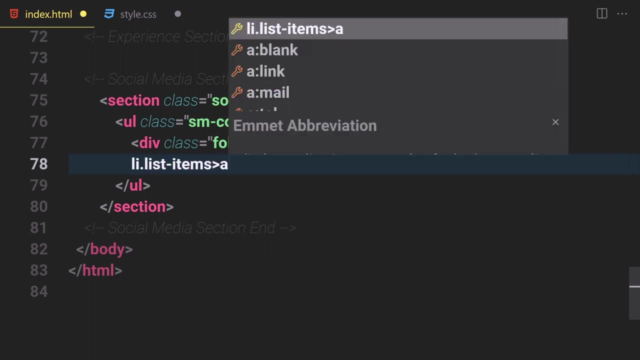 just use original with a class of follow. so this is going to be that kind of a grayish or whatever you want to call that color. so this is going to be that follow huge button. so we are going to be using li of list items. so inside each of these list item we will have our anchor tag and we want them to be like: 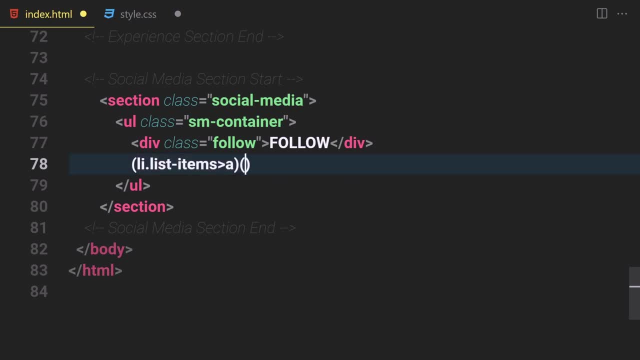 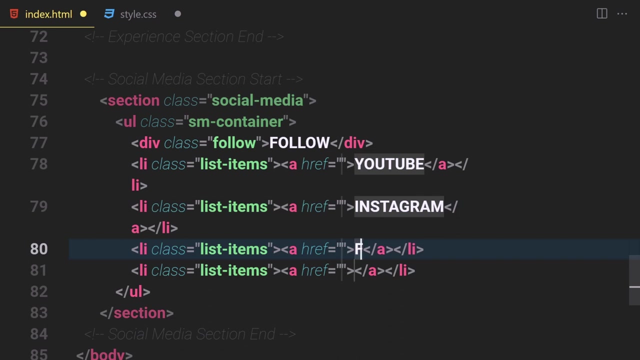 i don't know, so i'm going to use my image real quick. and, by the way, if you don't know what our image is, so you can check out my video on that, and we want them to be like four of them, so it will go to nowhere. first of all, we have a youtube, and then we have an instagram. it will go to a. 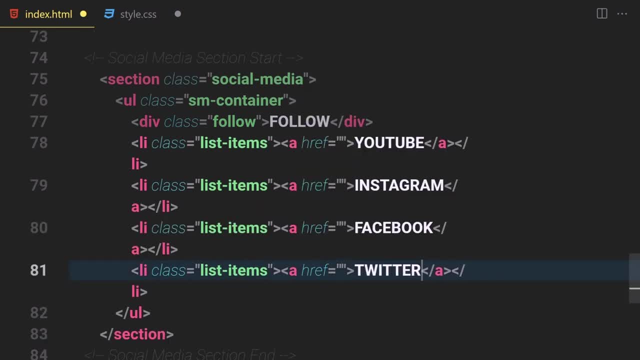 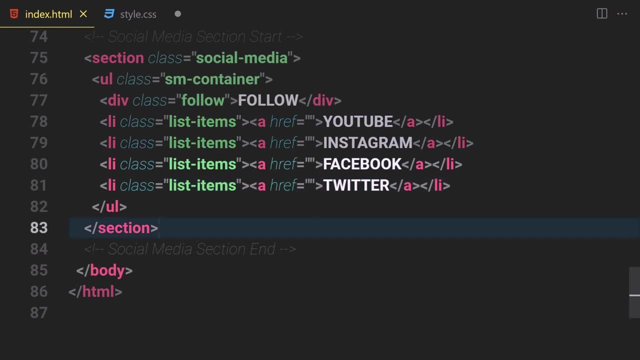 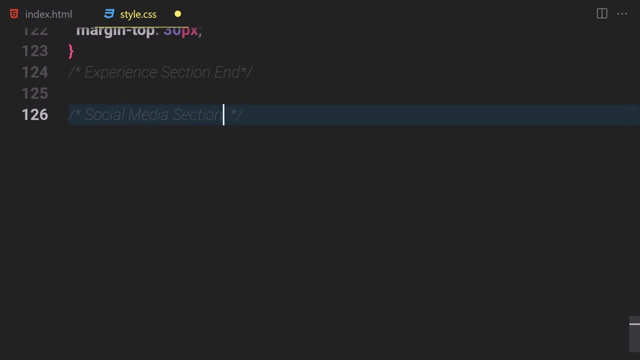 facebook. and then finally we have our twitter. all right, see if it's our file, and we cannot see that coding right away because it's hidden. so now let's just get into our css and now let's just try a little bit. all right, so i'm going to just write like a social media section start and then 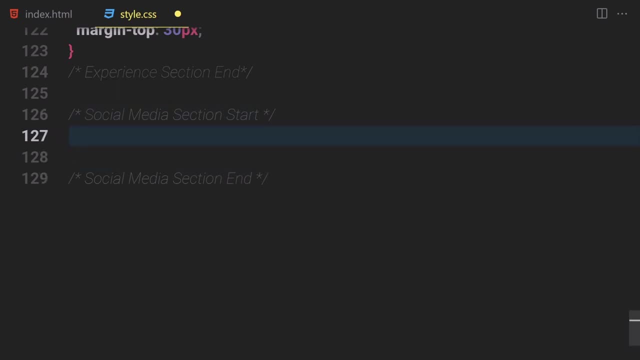 this is going to be the end of that social media section. all right, so what do we have to do in this case? first of all, we want to provide a margin. so social media. let's just select there which is this social media. let me just double check so that i didn't mess up with. 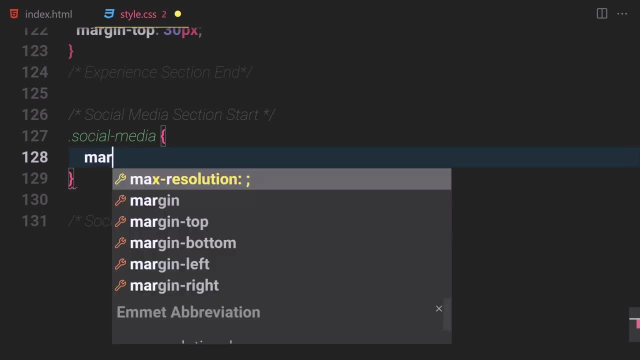 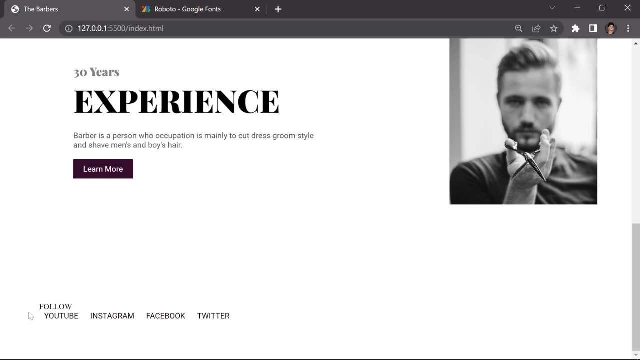 the spelling and let's just write a margin margin all around, like fireframe would be fine and i guess that would be fine. so this is how it looks like for now. i know it's looking awful, so we are going to be selecting there or we are going to be making cool there just in a second. so first of all, let's. 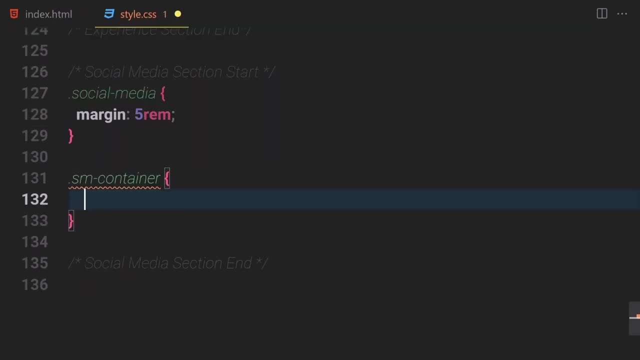 just select our sm container, which is that sm container right here. okay, so let's just use a display of totally flex. flex wrapping will be now set to wrap and justify content will be also set to center. align items will be also set to center and then text align. we are going to be using center. 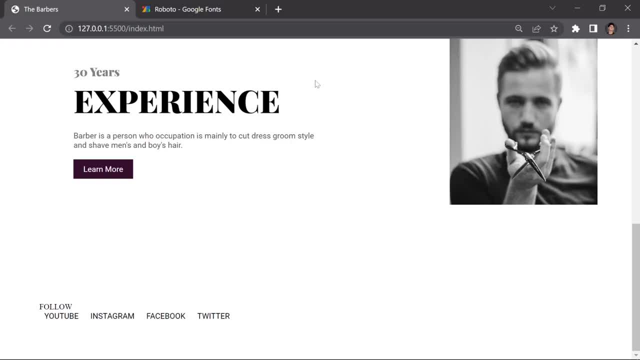 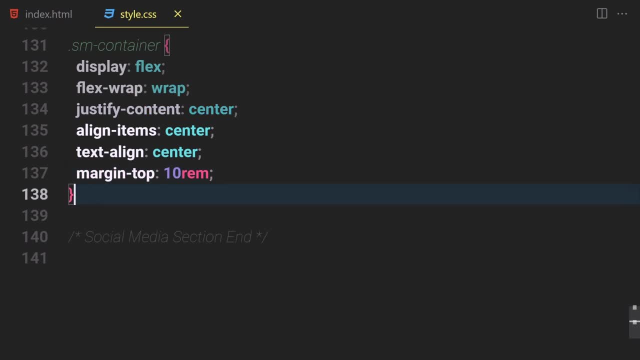 and margin for the top. we are going to be using 10 rems. so now, if you save a file and this is how it looks like for now, okay, so everything is perfectly centered, and so on and so forth. okay, so now let's just dial that follow button which we provide right here. so now let's. 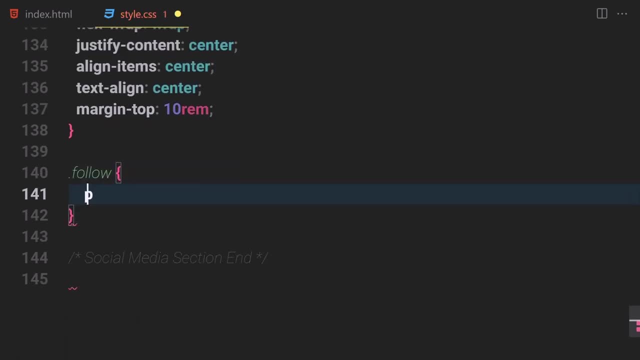 just select that first of all, and now let's just style that. so i'm going to use a padding of 20 pixel and i'm going to also provide a background margin to be that main color which we've, uh, declared above. so we are going to be using a color of totally white. a text color will be. 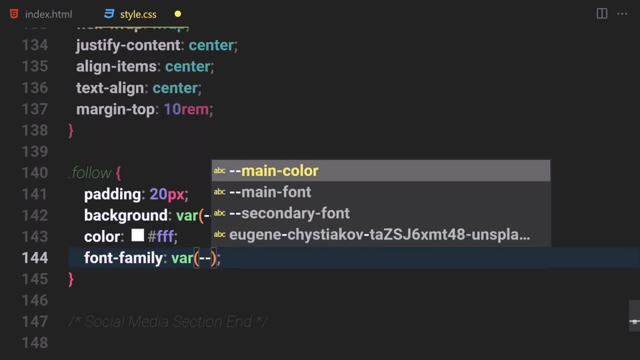 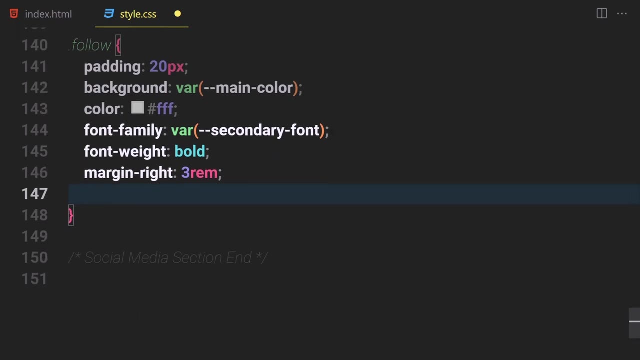 totally white. so we are going to be using a font family of that variable as well, which is that secondary variable or roboto. so font weight will be now set to totally bold and margin. i'm going 30, not 30, but three. why am i saying 30 all the time? so text alignment will be now totally set to. 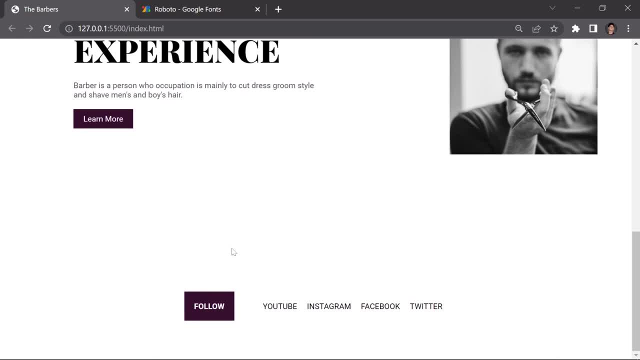 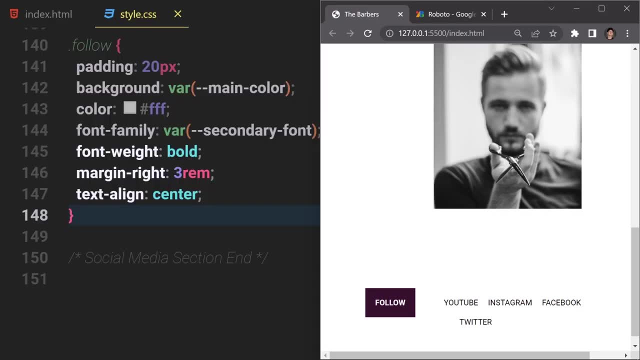 center and if you solve that, and this is how our button looks like for now. okay, so this is not a button, but it's kind of a label for social media anyway. so we are totally done with this section as well. if you want to change around, so feel free to do that, and we are going to be using media. 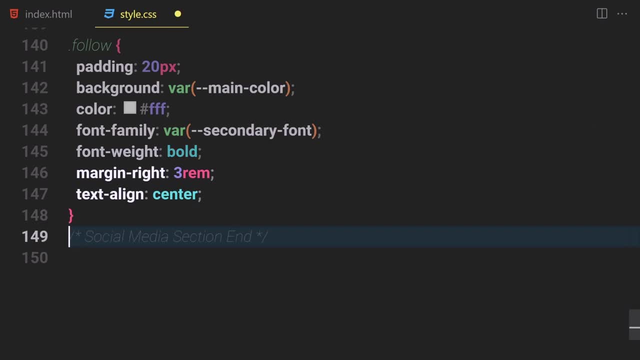 queries for that as well all right so we are totally done with the social media section what else do you have to do now let's just work on i'm just going to use the media and another ball pains action what we're ready to do next i'm going to use media query which will end the search � with 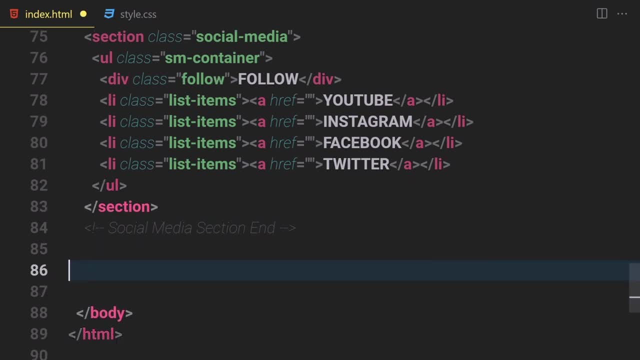 on topic settings and that is channel rating and that will be shown in your profiles. so, if all i way, so we have dry'm active, prompt, prompt, prompt. well, that's pretty much everything we have by all right, so we're just work on. or hero area, so i'm going to make it bigger and here we have to just write a section. 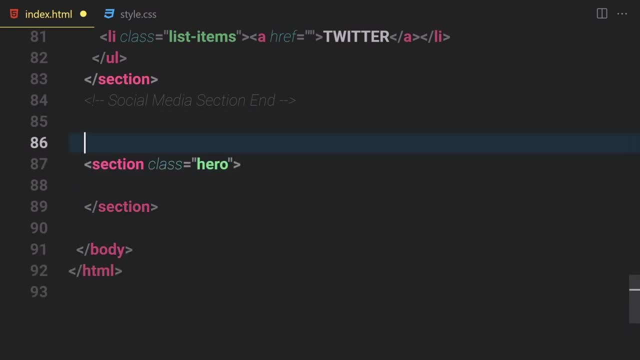 for or hero. so let's just write a comment for myself like a hero. oh my god, why is this getting replaced in here? so let's just use or hero section start duplicate. i want to cut that from here and i'm gonna paste it underneath this section. so here section and all right. so earn and start. 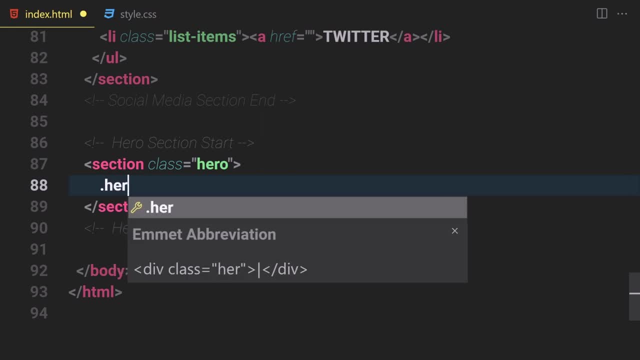 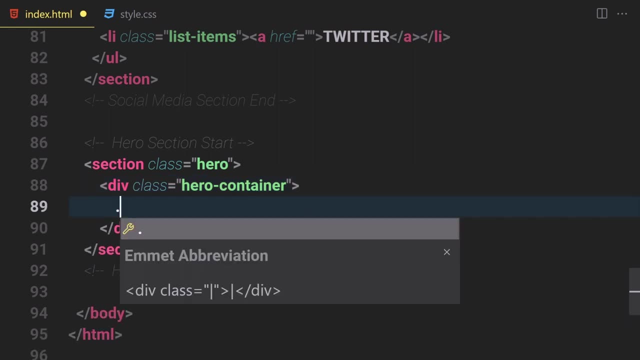 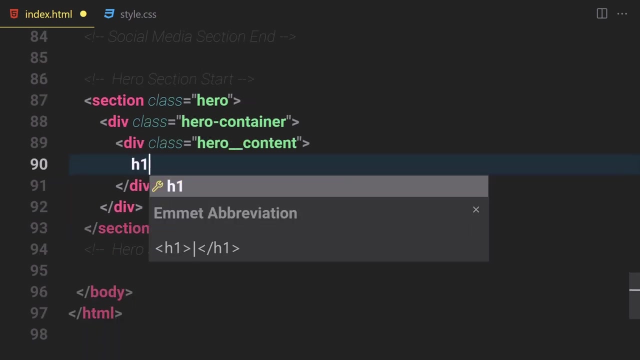 so inside this section, we are going to be using our div with the class of hero container. i messed it up: container like. so inside this hero container, we are going to be creating a new div with the class of hero and then content, content. so all of our content goes inside there and we are going to 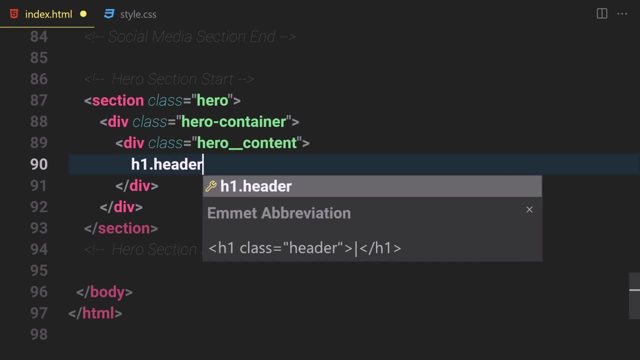 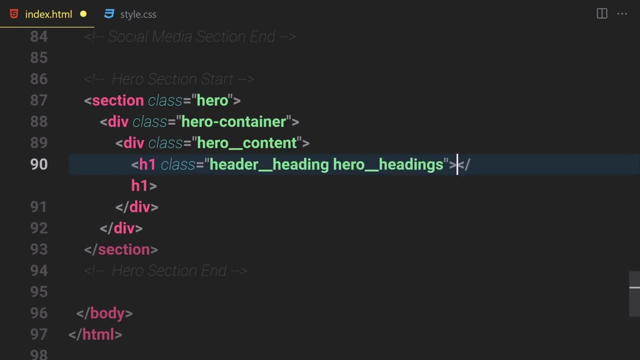 be using h1 with the class of header dash dash heading and we are going to be also also using hero dash dash. um, what head dings in this case? so we have a header heading and we have a hero. head dings, all right. so let's just write a meet and br or hero, so, or, uh, hero okay, like so. 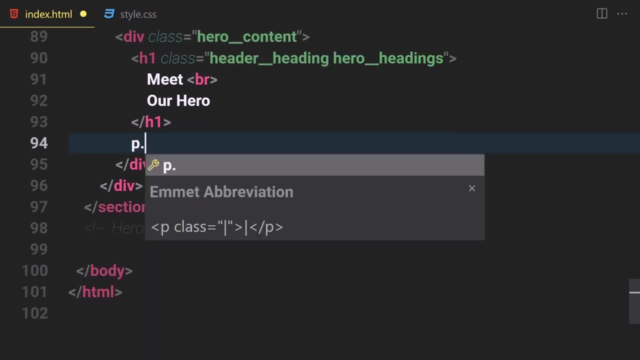 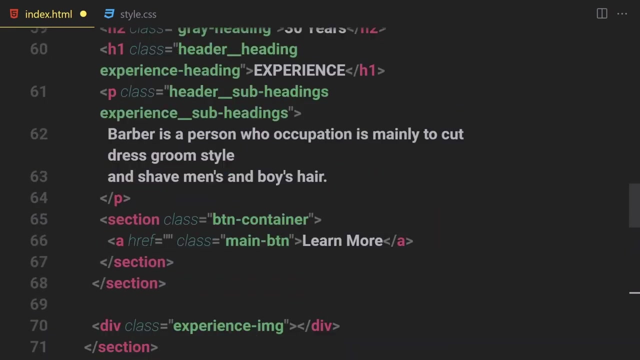 and underneath that we are going to be using a paragraph with a class of header and then dash dash, sub and headings. so we are going to be also using header and dash, dash, dash, dash, sub head dings. so inside this class we are going to be reusing that text again. so instead of writing, 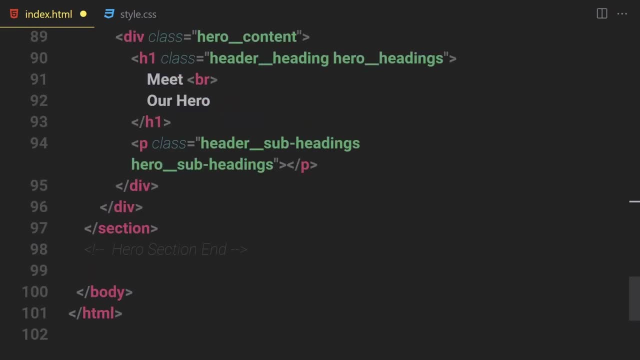 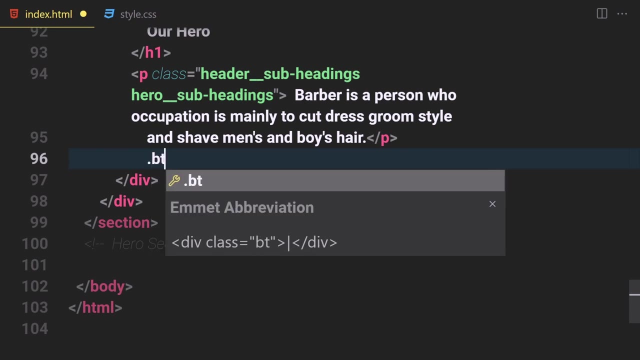 that lorem ipsum. i'm going to be using this text throughout this project. okay, so i'm going to paste that right here and outside from this paragraph. what do we have to do? we have to create a new container with a class of btn container and we are reusing that one more time. so we have a main. 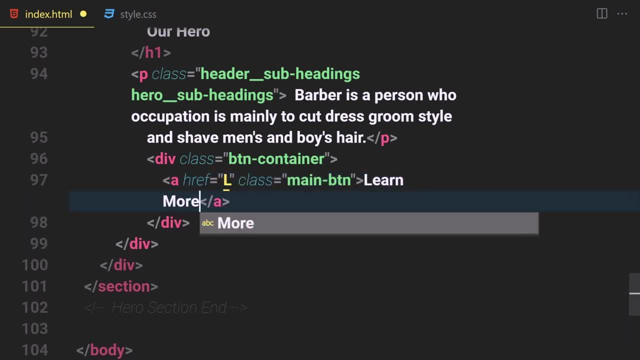 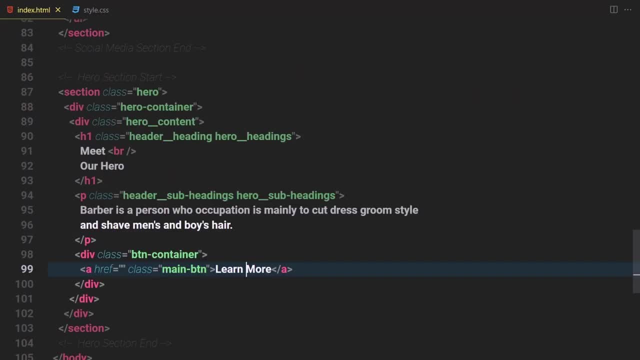 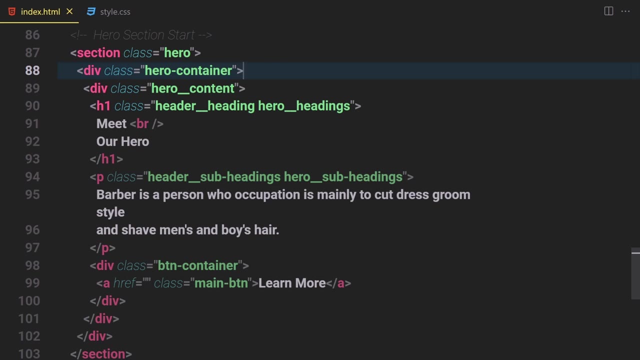 btn and learn, uh, learn more, and it will go to nowhere. okay, so nowhere. so if you save that, zoom back and this is how all of the coding looks like. so i'm going to zoom in a bit one more time. so we have a section with a class of hero, then we have a hero container. inside there we have a hero content container, then 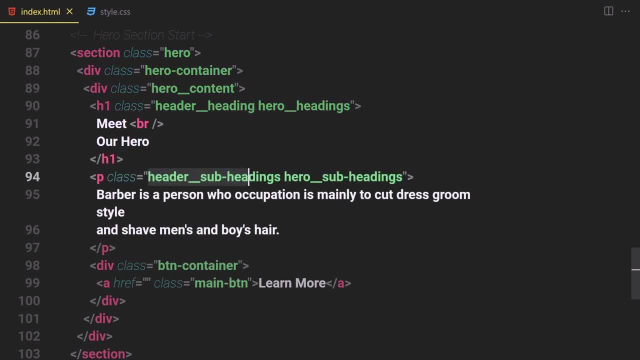 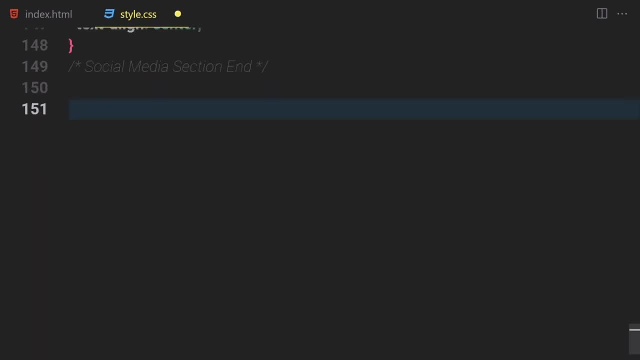 we have a hero heading, then we have a hero headings and we also have hero subheadings and stuff like that. then we have a button container, all right, so now let's just start working on that. so i'm going to zoom in a bit. so let's just select first of all, or hero section, and what do we have? 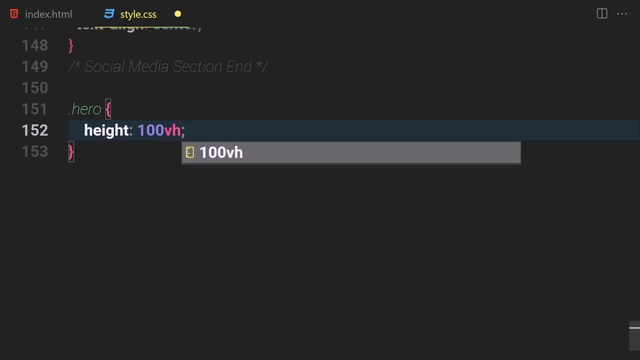 to do. i'm going to give them a height of 100 vh, so we are going to be also using a display of flex in this case. justify contour will be now set to center, align items will be now set to center and save our file. and this is how currently things looks like. all right, so now. 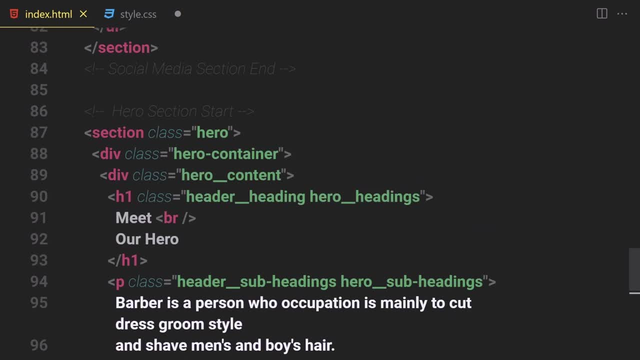 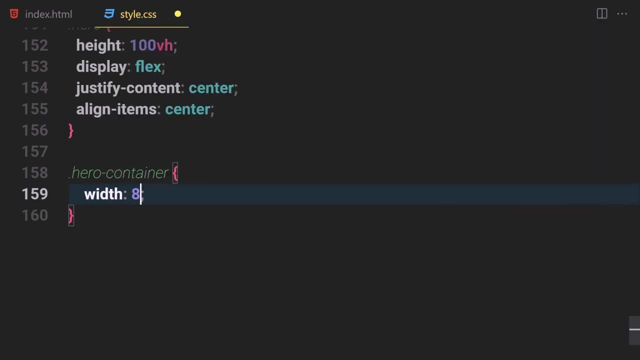 let's just select that hero container real quick. which is this hero container? so i'm going to copy that and i'm going to just select it in a second, and let's just give them a width of, like i don't know, 70, 70 percent- oh, my goodness, not 79, 70 percent. and i'm going to also give them a display of flex. 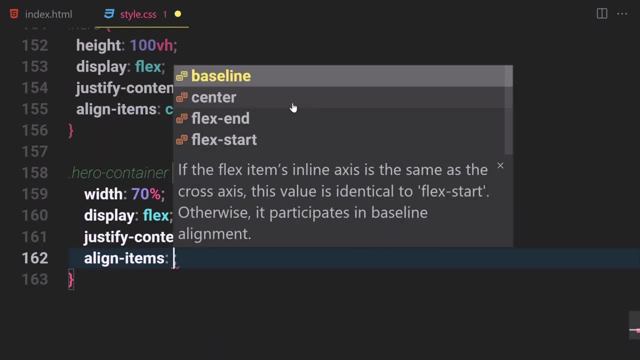 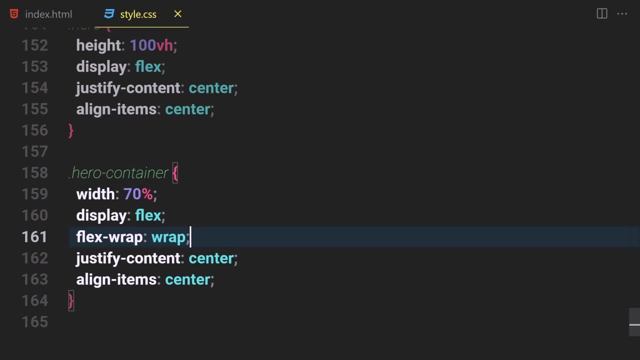 and justify content of center, align items of totally center, and yeah, i guess that would be fine for now. and also the flex wrap will be now set to wrap and save our file. nothing will happen for now, anyway. so now let's just select for hero image container. so we are going to be writing a. 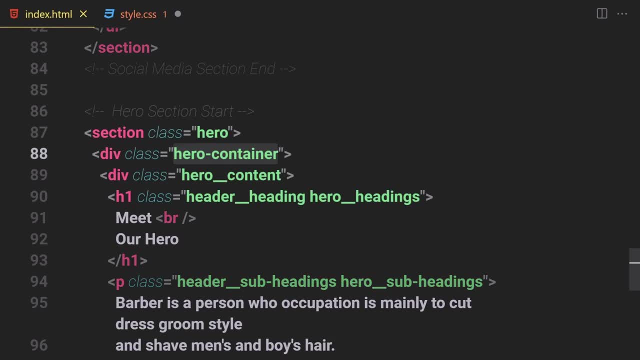 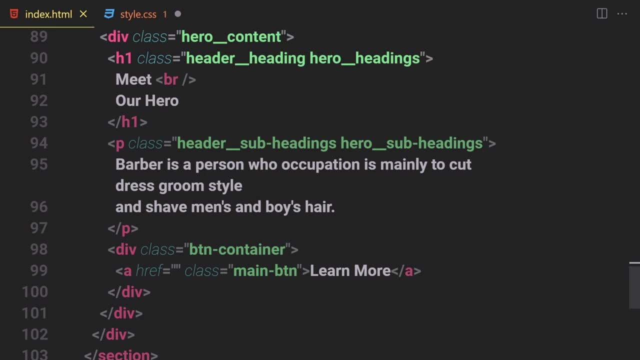 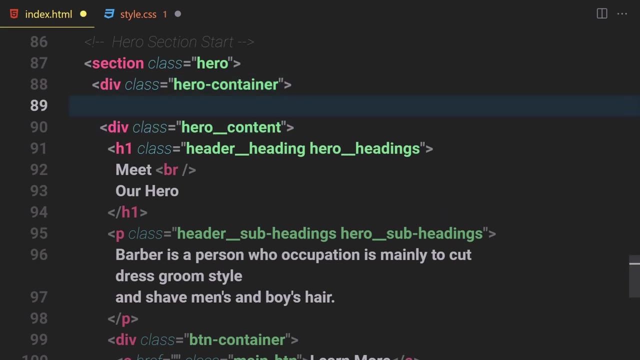 hero, then image, then container. so do we have a hero image container? i just brought a hero image container. i guess i forgot to include that. so we are going to be using this hero image container, uh, underneath this header, uh, this hero container. so we are going to be creating a new container for a hero: img and then container. 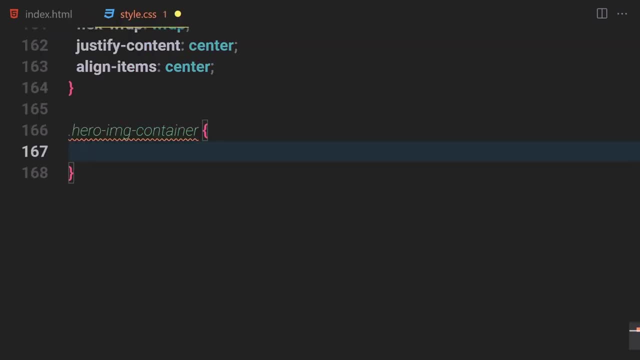 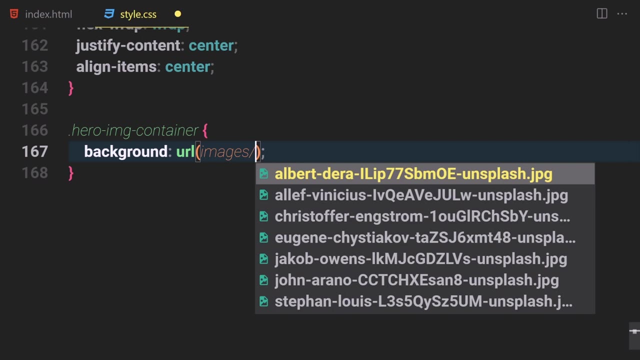 so this is going to be our hero image container. so now let's just style that a bit. so first of all, i'm going to use the background of our url function and let's just go to our images and select our albert this kind of person. so now let's just write a background size of what cover. 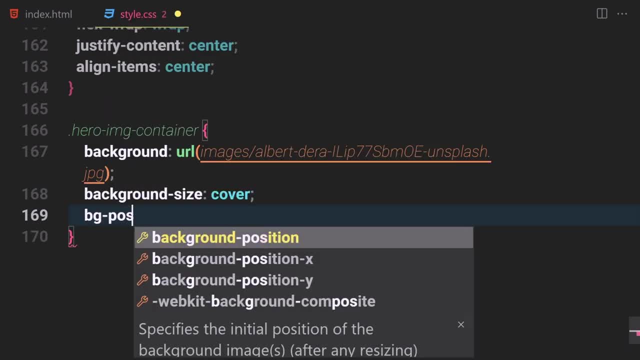 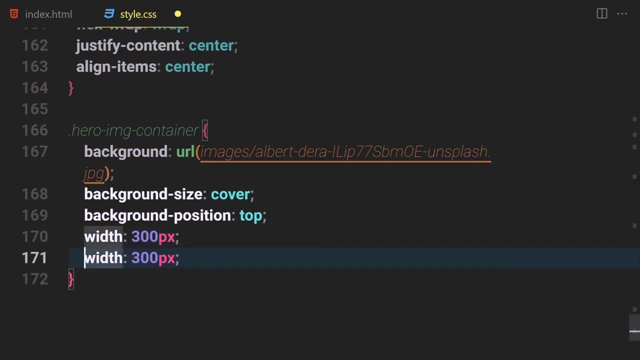 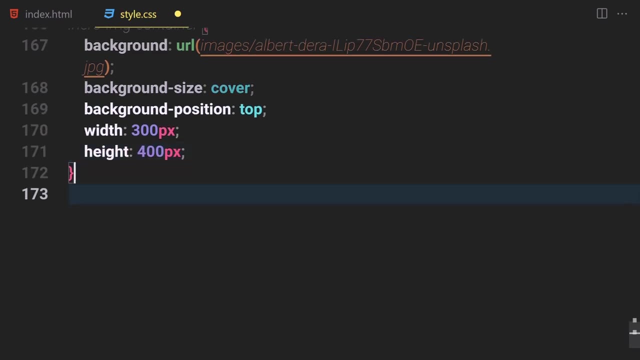 total and background position. uh will be now set to what top? and now let's just give a width of like 300 pixel and i'm going to also give them a height of 400 pixel in this case, so i'm going to just change that to a height. and also let's just select our hero and dash, dash sub headings which we provide. 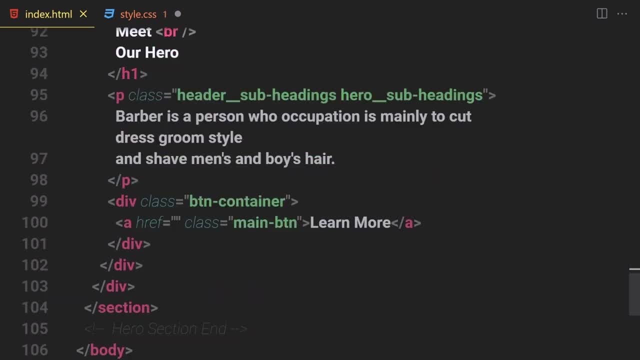 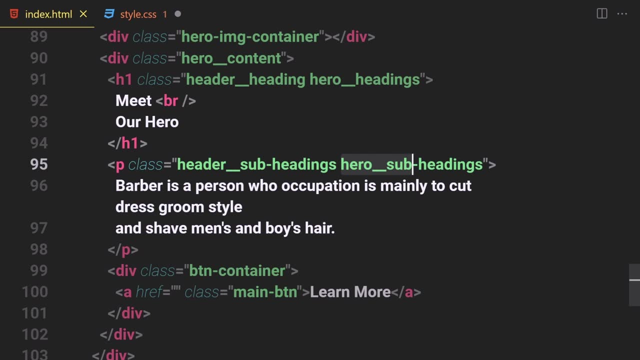 right here. so we give this hero heading clause, not this one, but we give a hero subheading clause and we also give a hero subheadings. i guess we have. so we have a header subheading clause and we have a hero subheading clause. right there, all right, so i'm going to just give a width of like 400 pixel in this case. so now, 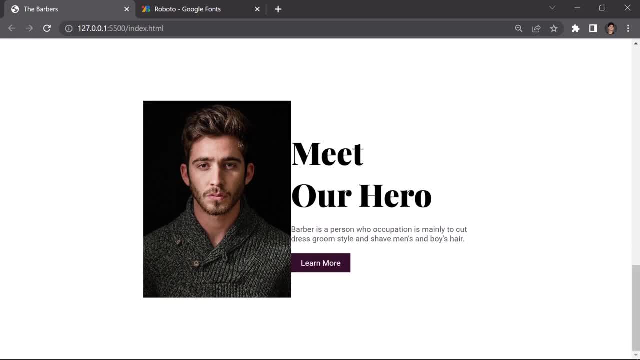 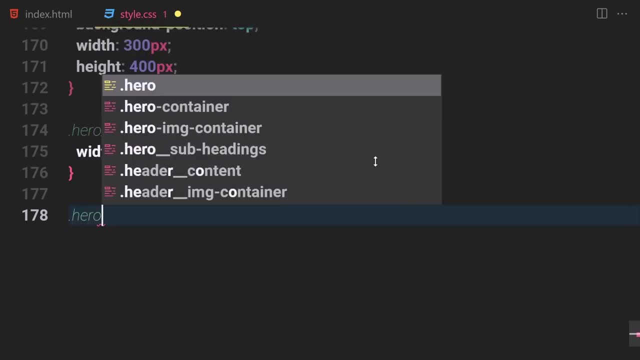 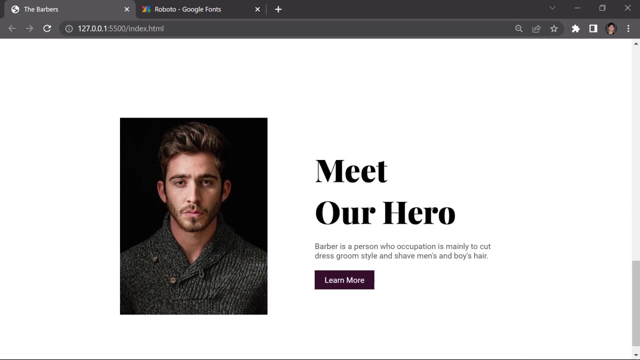 if you save that and this is how it looks like. so you know what. we need a little bit of margin for the left, so let's just select, or a hero, dash, dash content. so hero, dash, dash content. i'm going to just use margin for the left, like six rems. so if you save that and this is how it looks like, right, 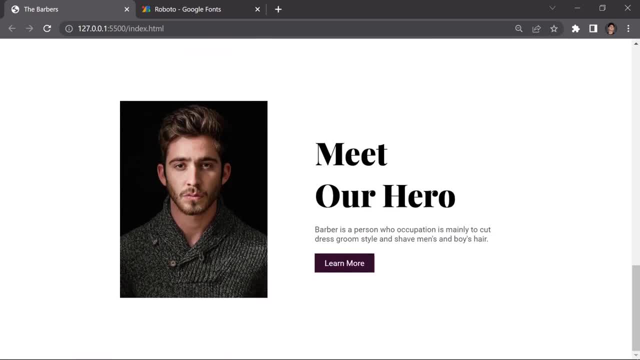 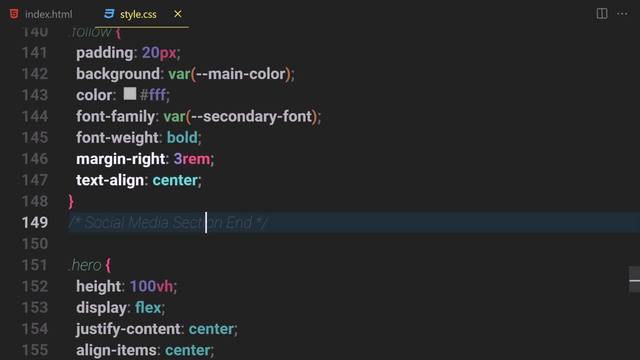 now, okay, so we are getting our hero subheading class and we have a hero subheading class right there in there. so now we are totally done with this hero section. so now let's just write or comment for ourselves. so i guess, uh, social media section n and let's just write hero section. 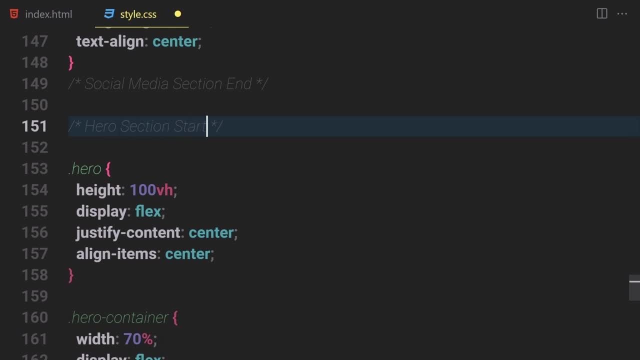 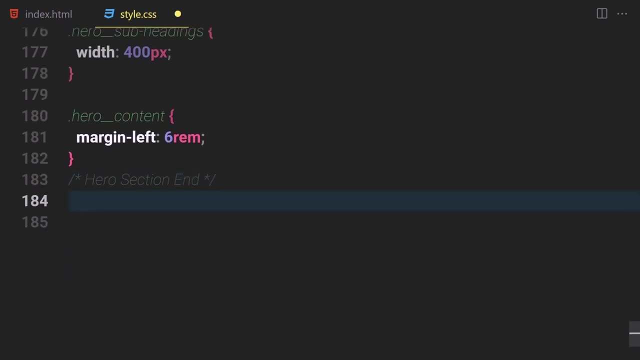 s-e-c-t-i-o-n. and then start, copy that and go to the bottom and i'm going to paste it right here and this one will be earned. so now let's get into a new section called services. all right, so underneath this section, or hero section n, we are going to be creating our new section with: 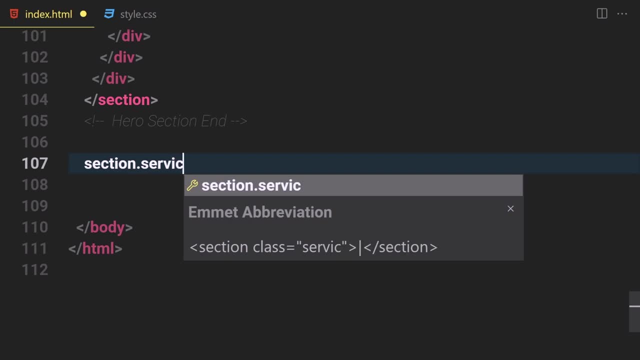 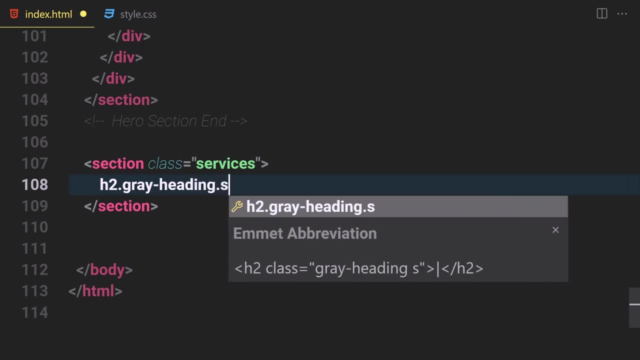 the class of services. so section services. so inside this services section, what do we have to do? we have to just write h2 with the class of gray heading and also services dash g, but not just dash g, but dash, dash g and then heading. okay, so we are going to be using like a top quality in. 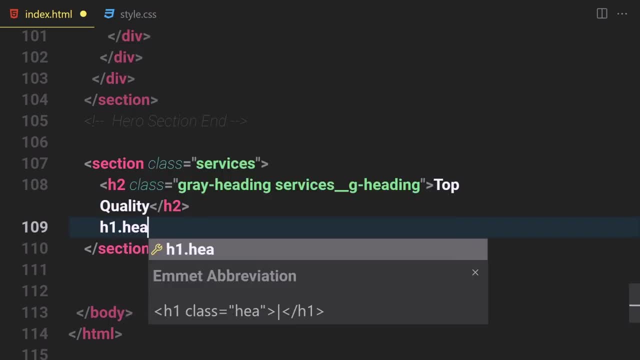 this case, and underneath that, we are going to be using our h1 with the class of header, dash, dash, heading, and in this case we are going to be also given a class of services and then services heading. all right, so now let's just put a label of services in here anyways. so now, underneath this, 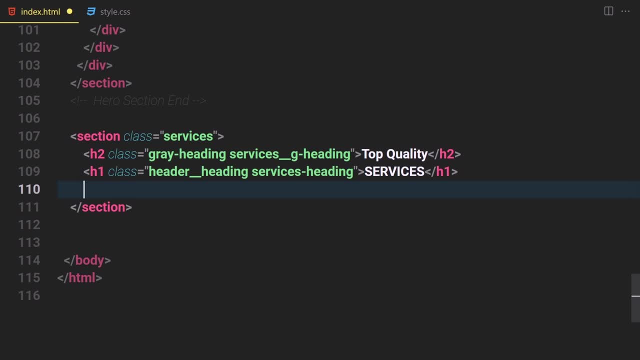 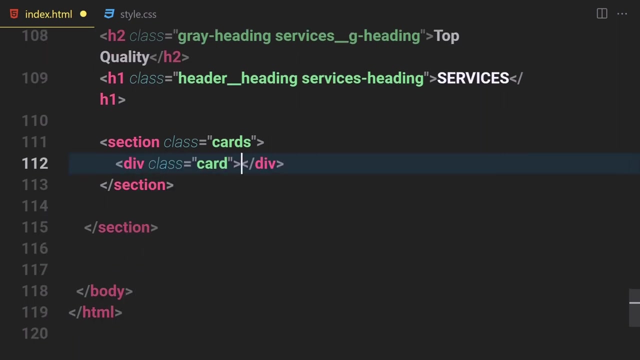 h1. i'm going to just zoom out a bit so you guys can see everything a bit better, and first of all let's just create our card section, so section uh, with the class of cards like a plural cards, not a singular. so inside there we are going to be using a few cards, so we have a card container one. 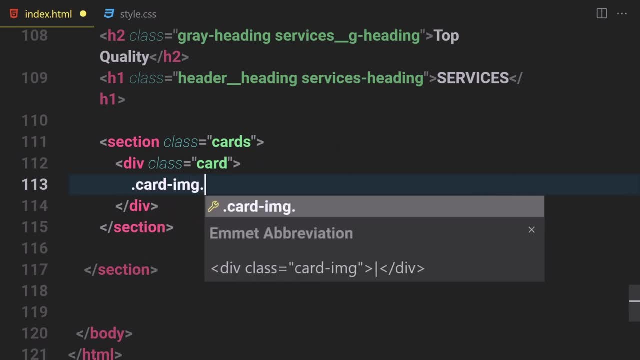 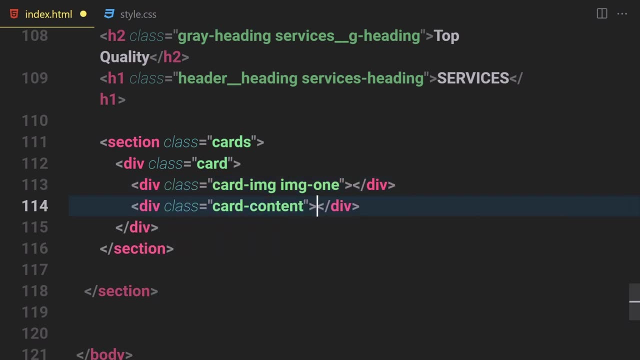 then we have a div: the class of card, img, and then img one. okay, so this is going to be the image for card and now let's just use a card content. so this will be the content of our card. so we are going to be using like h1 with the class of card title and this is going to be the title of our 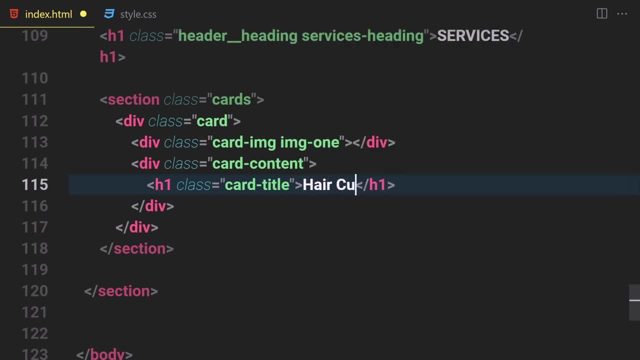 card. so i'm going to use, like a hair, h-a-i-r of cutting and now let's just write a paragraph with the class of card info and inside there you're going to be using or reusing that info one more time. so i'm going to 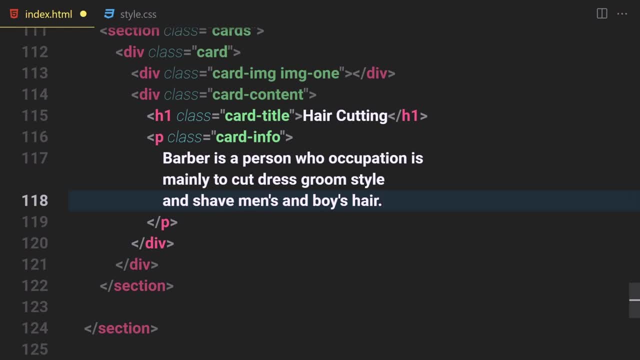 copy there real quick and i'm going to paste it right here, okay, so groom style would be fine. so instead of writing and shaving and stuff, i guess that would be fine. and underneath this paragraph you're going to be using anchor tag with a class of what main- btn, and also the card, btn. so 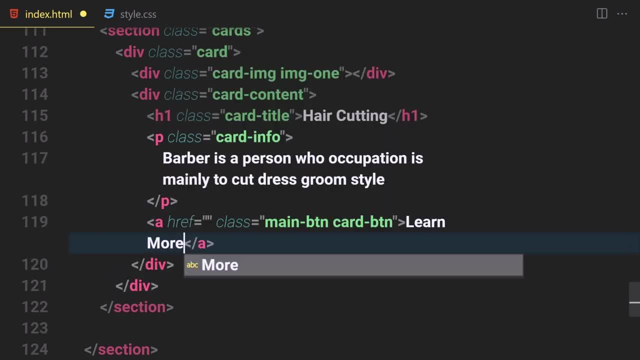 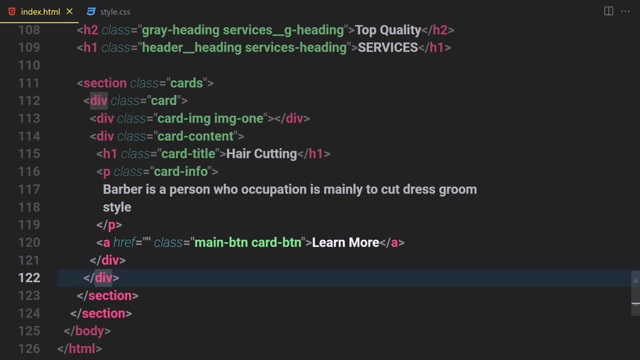 here. you're not going to be going to anywhere, so let's just put a lorem, not lorem. if some learn more and if you sell that, so this is going to be our first card. so let's just click on here. so it will now select right here. i'm going to select this first card and i'm going to use it. 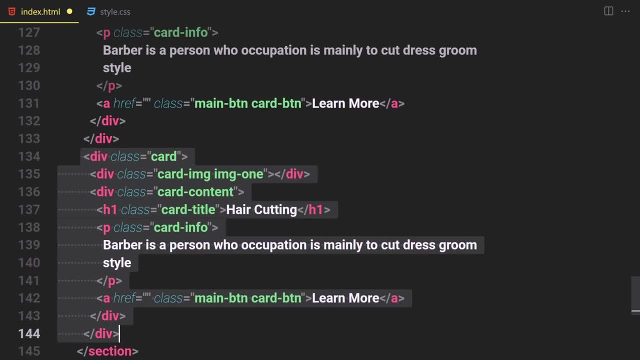 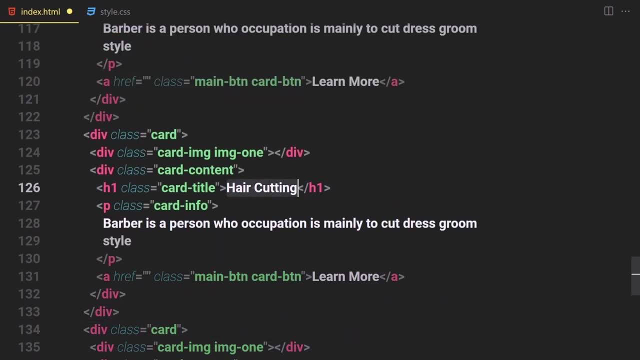 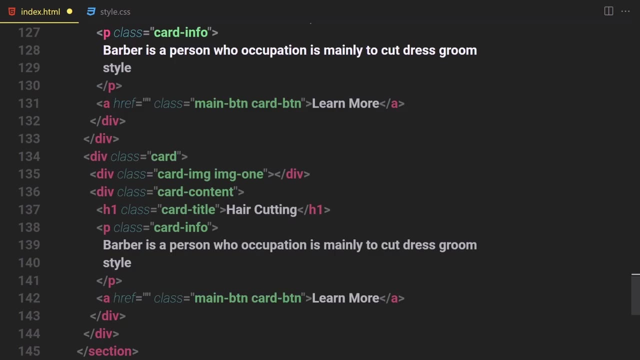 like two more times. so this is going to be the second, and then the third, and now let's just change the content inside there. so this is going to be for hair cutting and this is going to be for beard trimming, so beard trimming, like so, and i guess the other stuff will stay the same, and this: 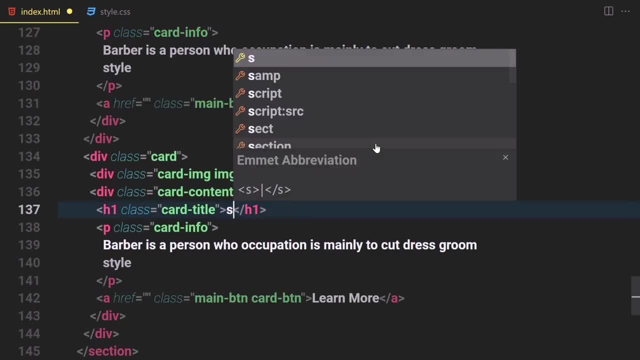 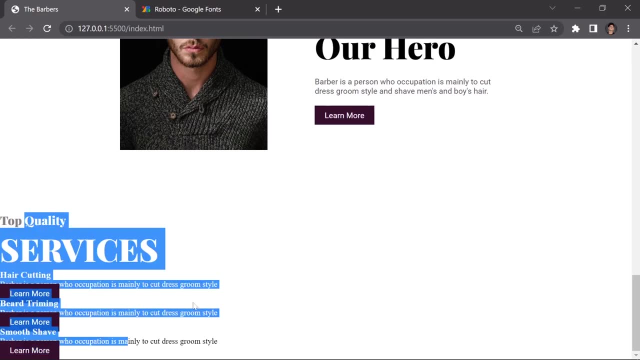 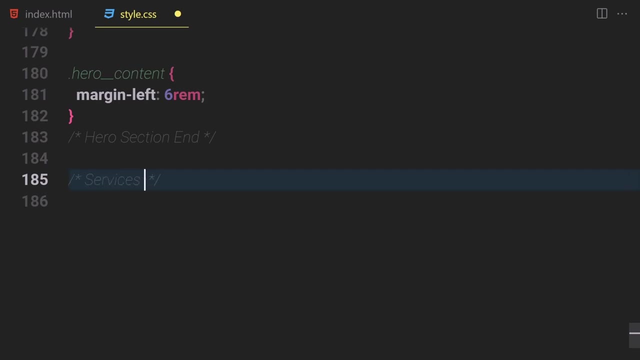 is going to be for what this is going to be for: smooth shave, so smooth shave like so. so if you sell that and this is how currently things looks like right now, i know it's ugly. now let's get into our css and knowledge style or services section, uh, section, start duplicate then this: 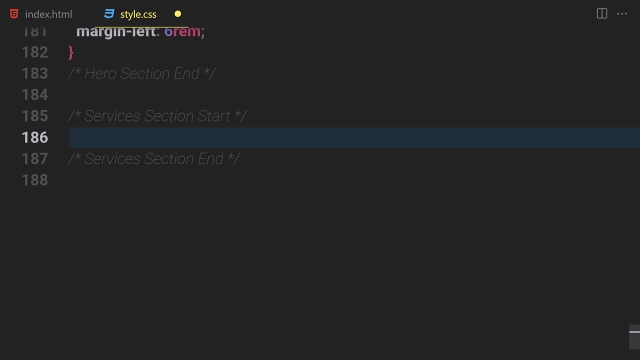 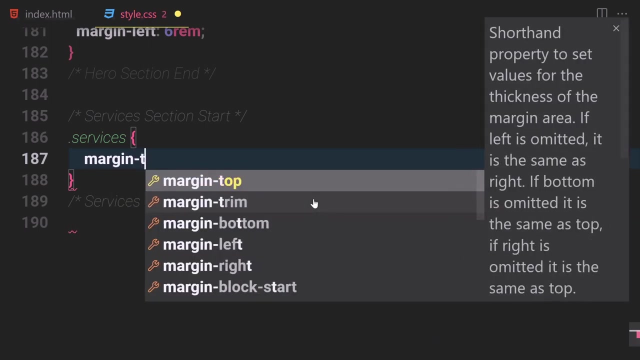 is going to be the end of our services section. all right, so now let's just start working on styling. so what do we have to do? first of all, i'm going to select my services section right here. for the margin top, i'm going to give like 10 ram, okay, so let's just 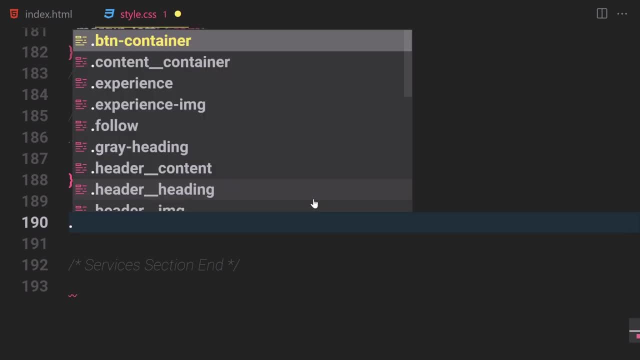 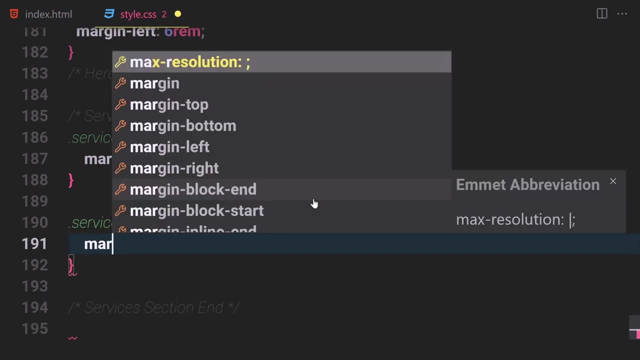 write a quote a little bit fast because i know this video is getting longer. so services and also that g. so i guess that was a dash dash g of heading. i'm going to give him a margin for the left, and margin left will be now set to five frame. and now, if you save that, this is how currently. 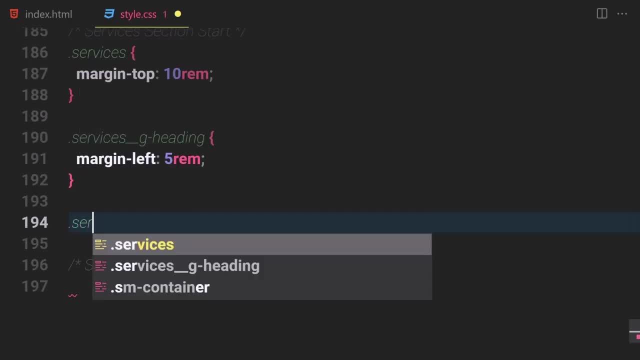 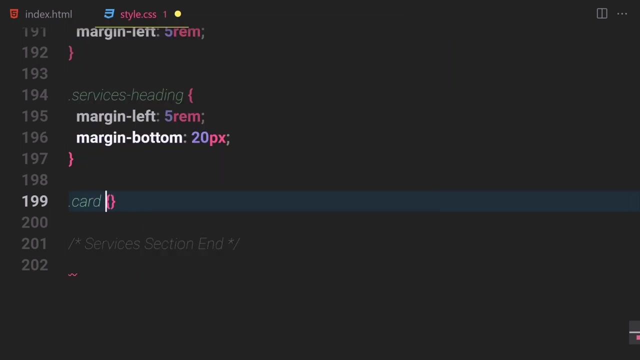 things looks like. and now let's just select our services section heading. so services dash heading. i'm going to give a margin left for like five frame and also the margin bottom will be now set to 20 pixel. all right, so knowledge style or card section. so first of all i'm going to select my 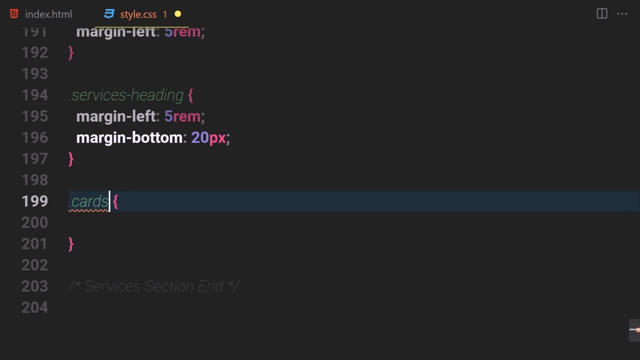 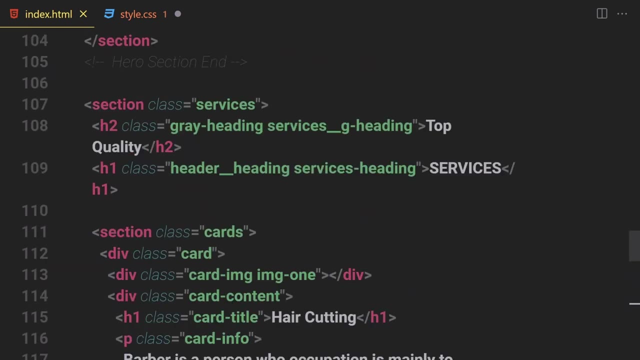 card, just a regular car, or you know what we are going to be? first of all, selecting our cards, like a plural uh, which is this one. let me just show you there real quick. so we've got one car, two car, three card. we have this card section right here: not a card, but a card. so now let's just select. 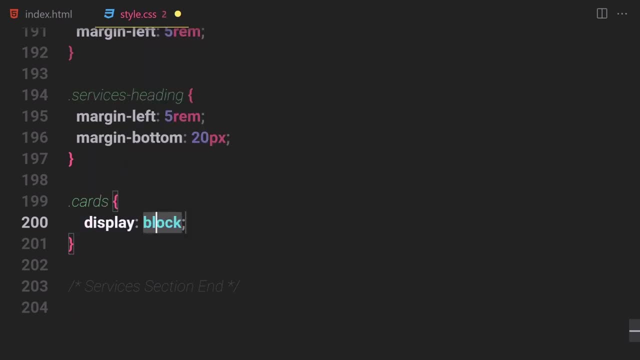 that, and now let's just dial that up. so what do you want to do with this? so we're going to select our card. so first of all, we are going to be using a display of flex on it and then flex wrap everything we want them to be wrapped. so justify content will be now set to totally center and 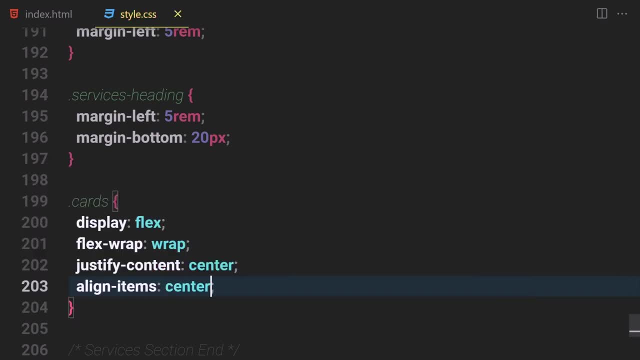 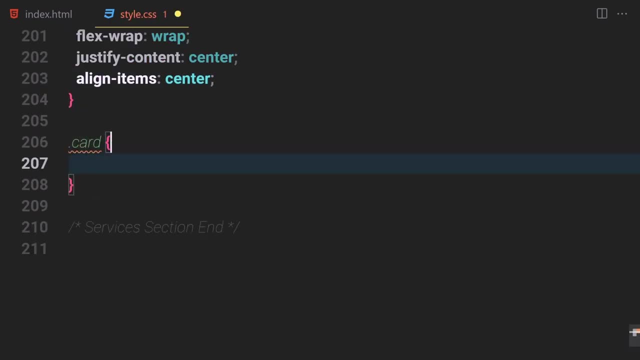 align items will be also set to what center now, if you save a file, and this is how currently things looks like. all right, so now everything is now totally at the center. now let's just select each of the card. i'm going to give them a width of like 300 pixel, duplicate that and change that to like. 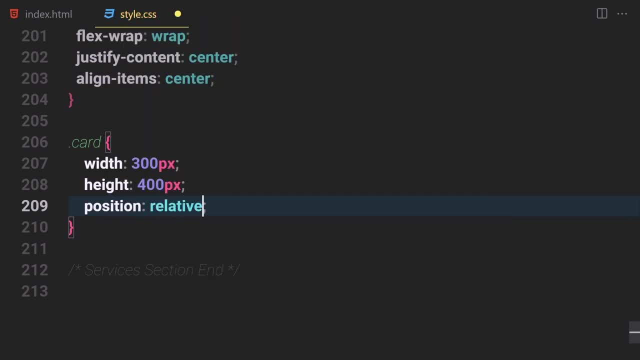 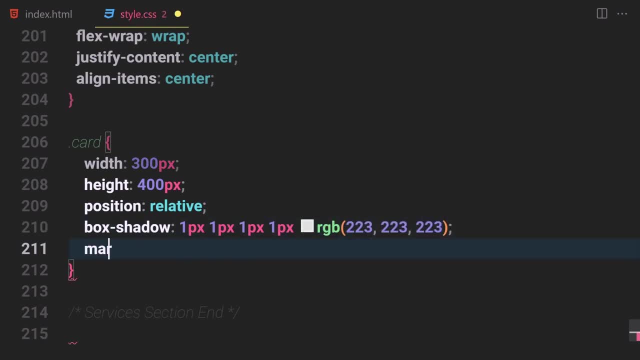 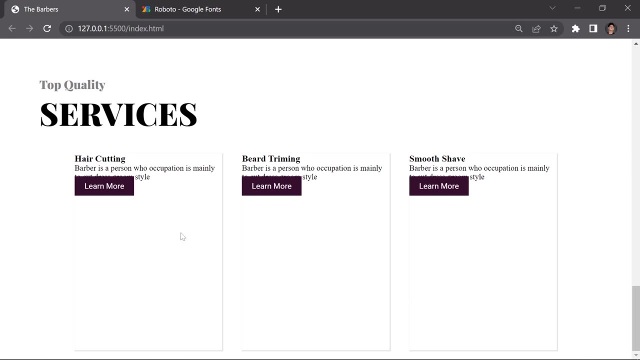 three, two, two, three, two, two, three would be fine, all right, so i'm going to just provide a margin of 20 pixel all around, and now if you sell that, and this is how you can see there, so no, so width will be 300 pixel and height will be 400 pixel, and we just provide a little bit of box shadow to it. 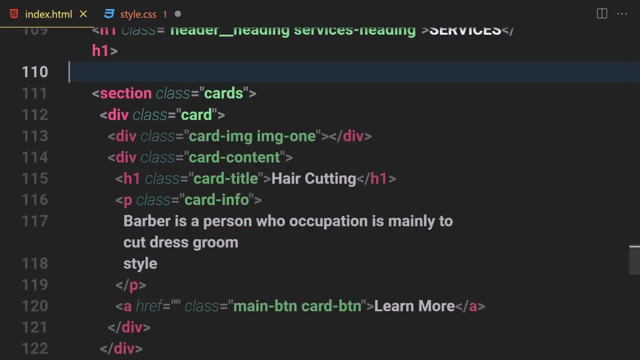 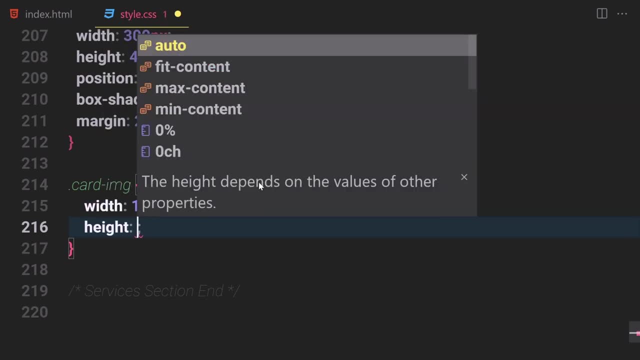 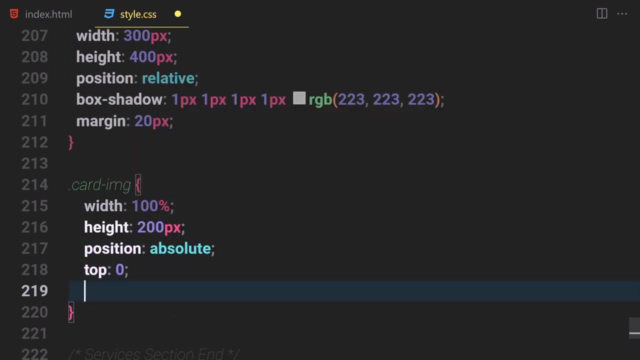 anyway. so now let's just select our card image. so which is that card image? so we provide that class to each of the card we are going to begin with of like 100 percent, and height, in this case, will be now set to 200, pixel position will be now set to totally absolute and top will be zero. left will be 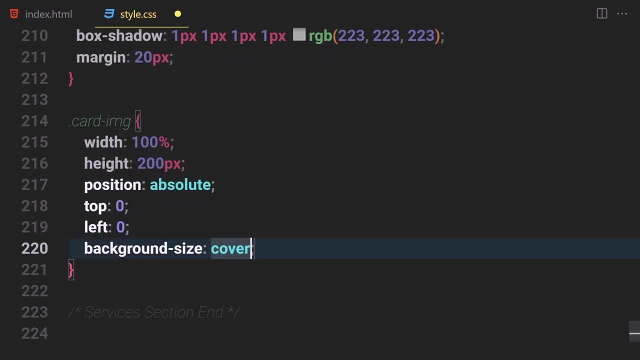 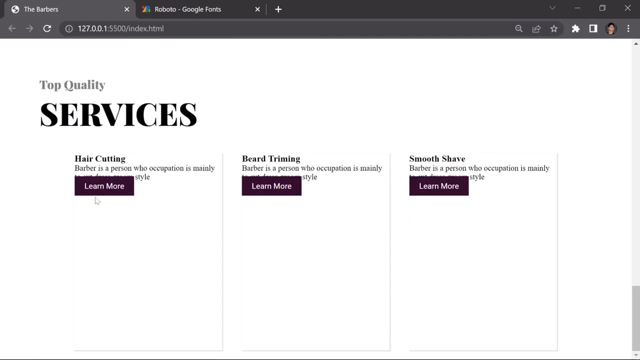 also zero. so i'm going to just provide a background size of totally covered, and background position in this case will be now set to top and if you save that, let's just see all right, so we cannot see anything thing. so now we can select each of our card and we can specify different kind of images for that. 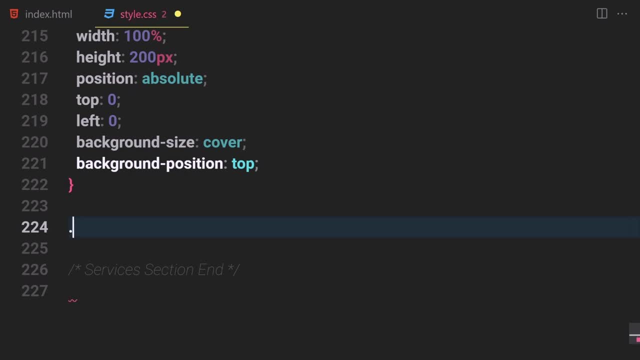 so, first of all, what do we have to do? i'm going to select my image once. so i'm going to just write like: img, dash one. so if you just write that, then i'm going to just provide a background, not a color, but an image. so, background, image. i'm going to provide a value of url. i'm going to go to: 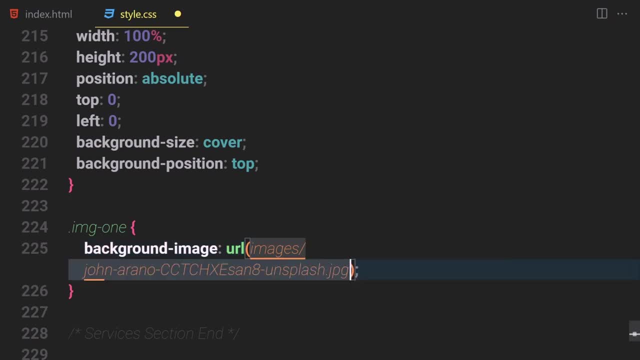 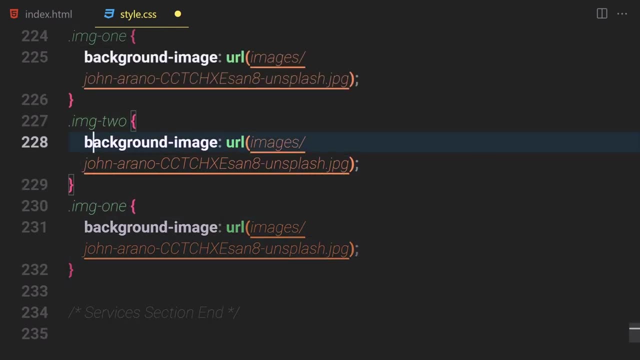 the images folder and we are going to be selecting or john and that first image. so now let's just duplicate that three times, and not three, but two times, and this is going to be now the second one. change the image to something else. so, uh, let's just select like lf or whatever the 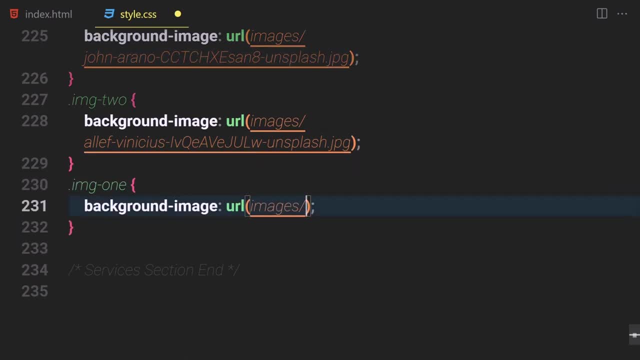 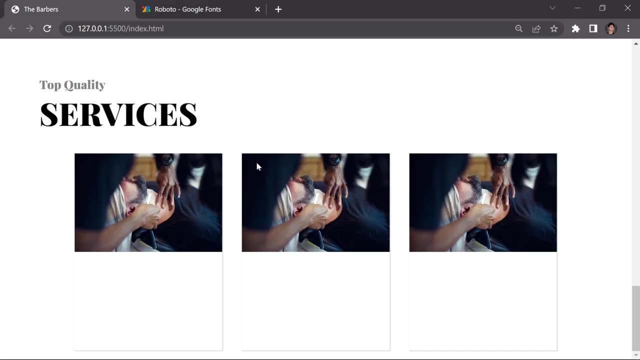 name is, and now let's just select the other one, and this one will be now christie. sorry, i can't pronounce the name of it. so now, if you save that, and now let's just wait for it. so here you can see the log uses all of these images right here, and i'm not sure if all of them are the same. 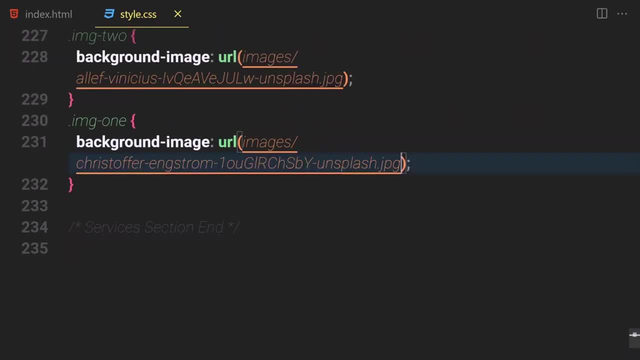 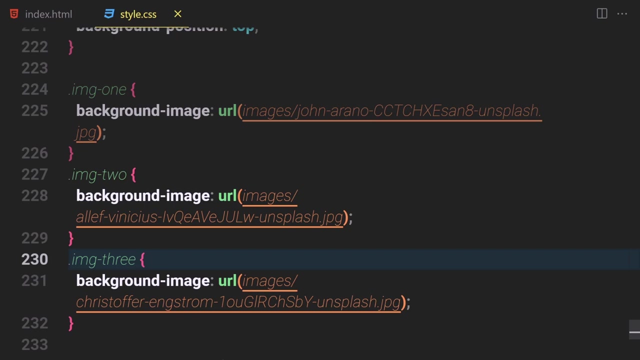 images or what's going on. so we've got image one, two and this is going to be a three. so image three, let's just wait for it to render. uh, okay, something went wrong. so we have img1, img2. this is going to be the. what is that? img1, img2 and img3. let's just see. 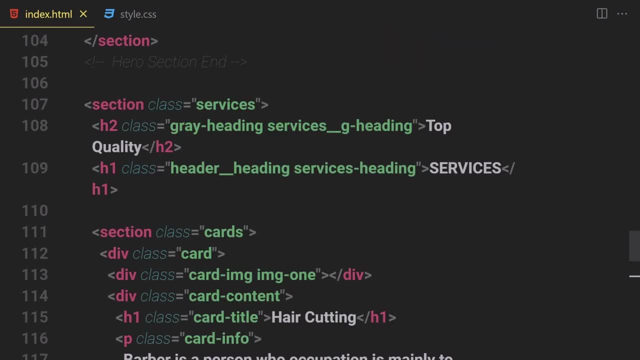 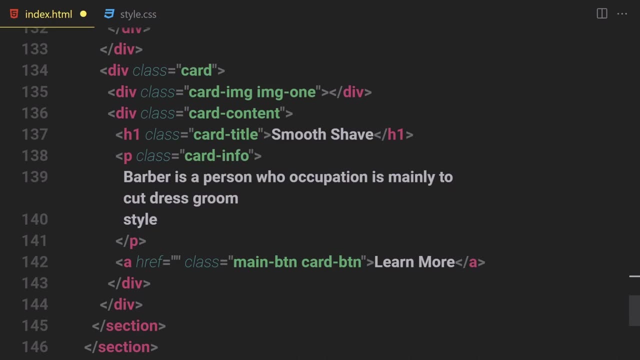 so we've got arts. we didn't change that. so this is going to be, uh, image one, this is going to be the image two, and now let's just check this one out. and this is going to be the image three. so project one. so we've got mid-term for image two and image three. we've got image one: two birds. 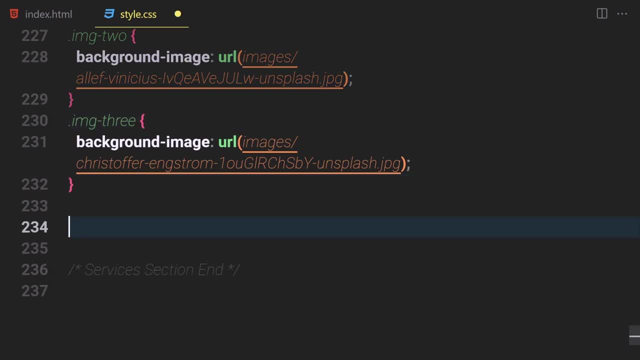 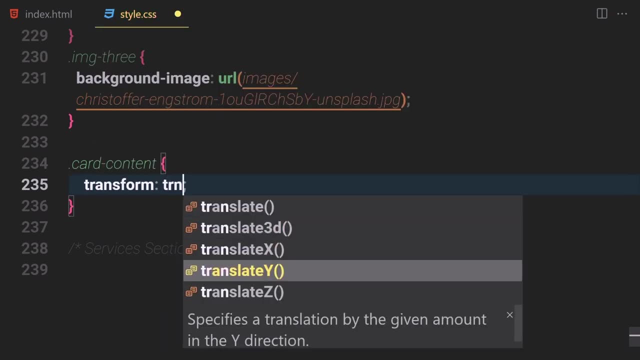 and we need to restore that image for our image. so we will now get totally different results right here. all right, so now let's just get into it one more time. and now let's just select that card content first of all. so we are going to be selecting that card content, and now let's just 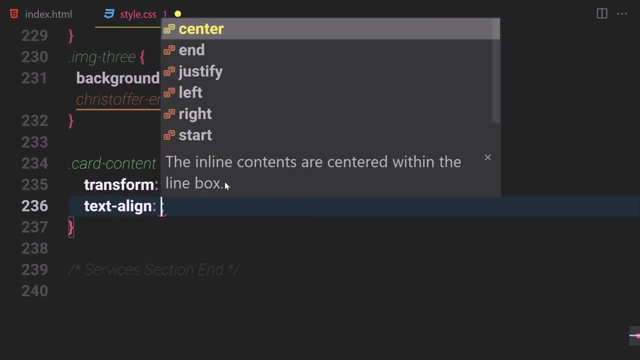 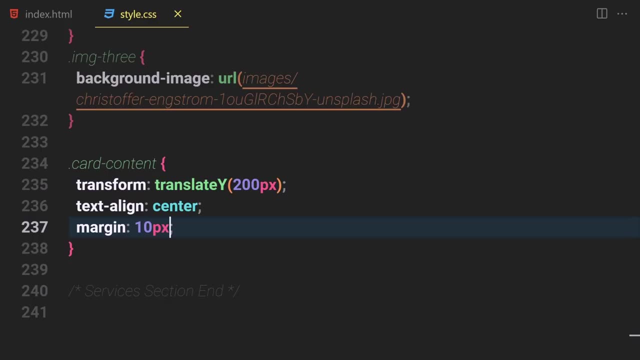 provide a transformation and it will just translate. it will not just translate itself to like the yx- yx is uh- will be 200 pixel and the text alignment will be now set to center and margin. i'm going to. so what else do we have to do now? let's just style that car title real quick. so we are going to be. 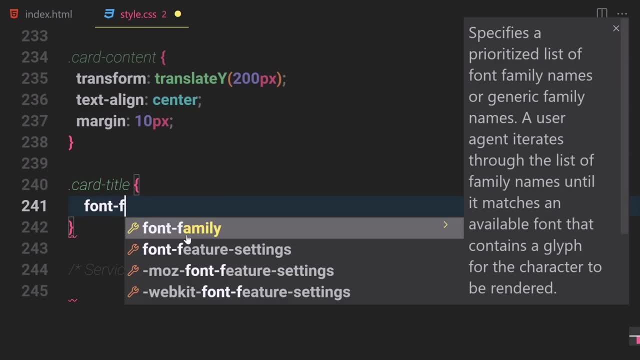 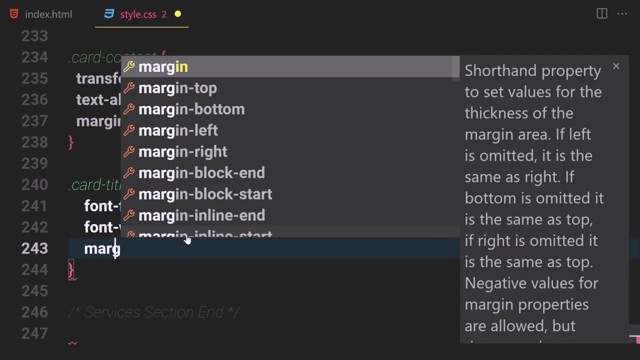 just selecting car title, and let's just provide a font family in this case. so we are going to be just providing, like, a sensor for to be fine, and font weight will be now set to totally normal. i'm going to give a margin for the bottom, like 20 pixel for top, and you know what? uh, i'm going to. 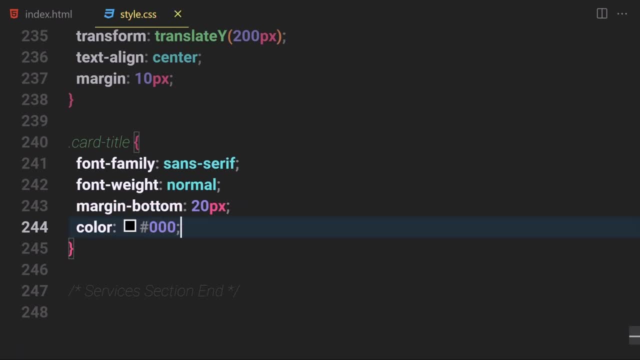 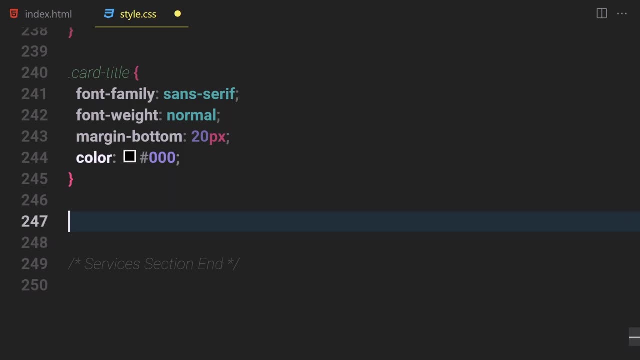 just give a margin of 20 pixel and color will be not totally black. and if you save that and this, how it looks like right now, all right, so that was a car title. now let's just select the car info, like these info, these text, right here. so now, if you just write like car info inside, there we are. 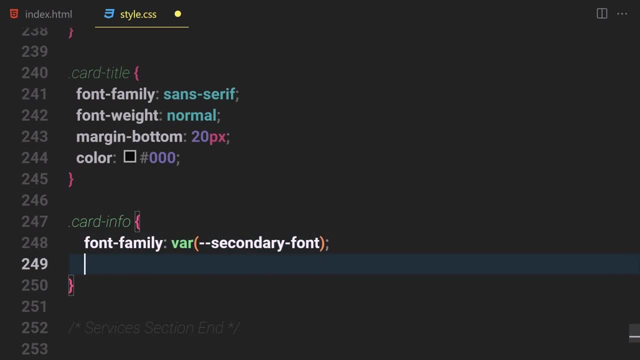 going to be using a font family of war or secondary font, and the text alignment, in this case, will be now set to center, and i'm going to change the color to be like: um, rgb of 109, and let's just write 109 and 109 in here. come on 109, and this one will. 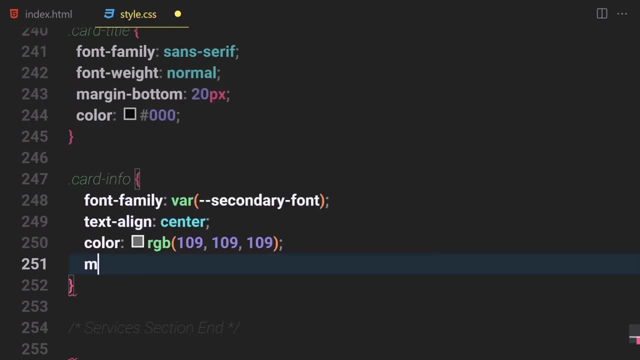 be also 109. all right, so now let's just provide a margin. for the top and bottom will be 30 pixel and for the left and right. let me just select that for the left and right will be 40 pixels. knife is our file and this is how it looks like right now. so we are now totally done with the 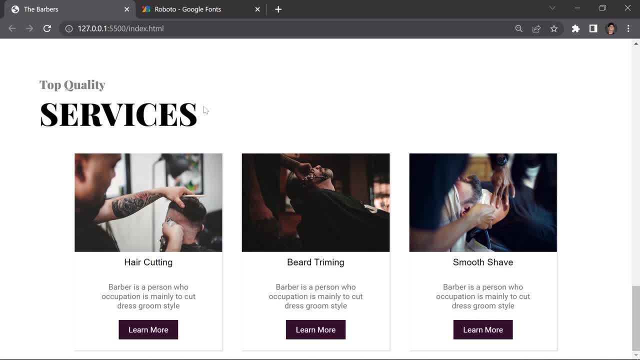 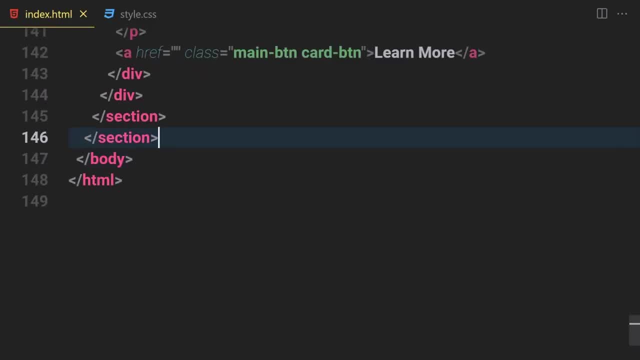 services section as well. so now let's just start working on our photo area. so this is going to be the last area of our project, so we are going to be working on a photo, all right. so for html, i'm going to just come here and inside that section i'm going to just write a comment for myself, like: 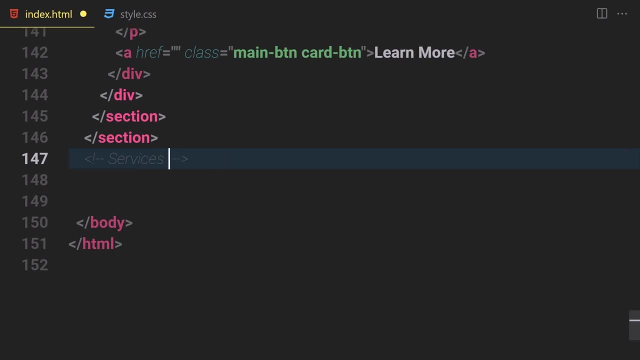 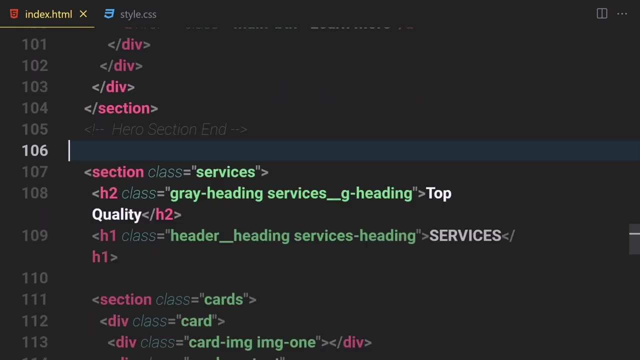 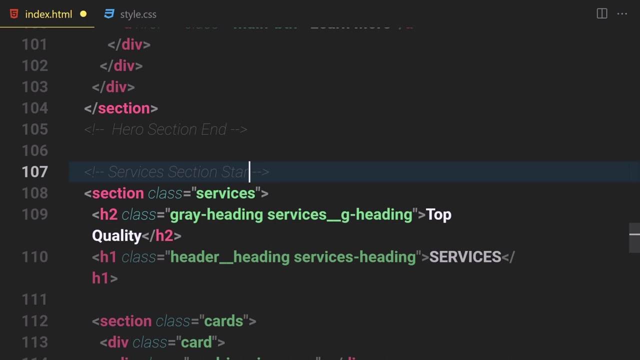 uh, services section s-e-c-t-i-o-n-n-n. i guess i write that somewhere in here. you know what? this is a hero section. so let's just write a services section s-e-c-t-i-o-n and then start go down. and now let's just start working on our photo area. so i'm going to write a photo. 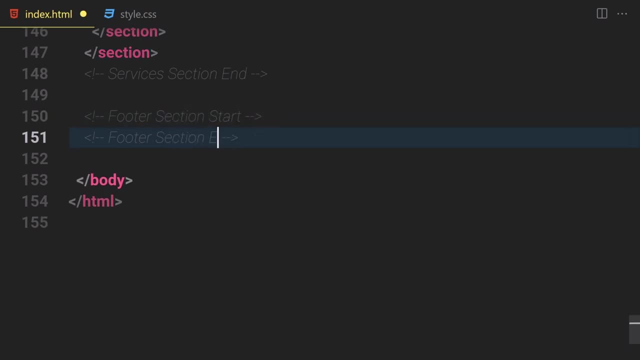 uh, section, uh, start, and now let's just duplicate there and end. so what do we have to do? we are going to be writing a photo with a class of folder and inside this folder we are going to be writing a div with a class of folder- dash, dash card, so lowercase card. and now inside that we are going to be writing: 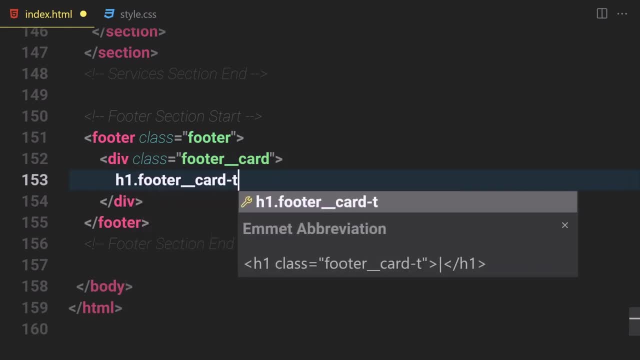 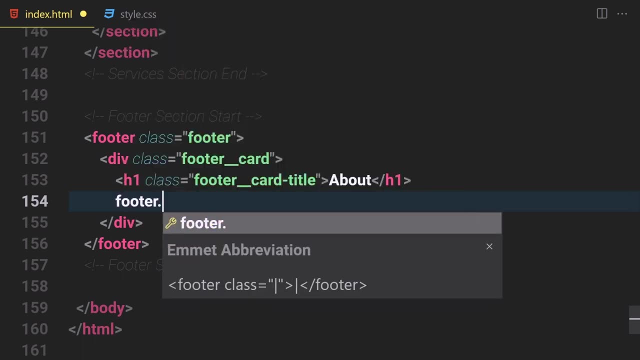 h1 with a class of folder, dash dash card, and then dash title, and the title will be about in this case: and now let's just duplicate there, or you know what we are going to be: first of all writing a folder and then dash dash card. i'm going to have to write a comment in there and then 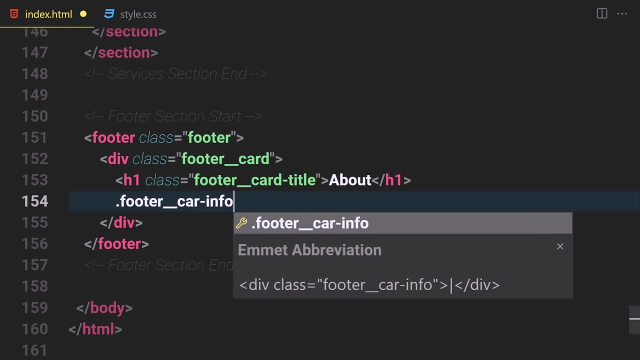 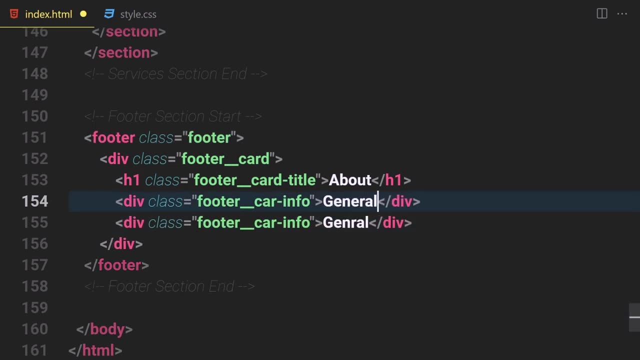 not a comment period. so card and then dash info and hit tab. so this is going to be like a general duplicate there. uh, this is going to be g-e-n-e-r-a-l like a general. uh, all right, so now let's just write our traffics. uh, duplicate this one more time and f a q. okay. so what do we? 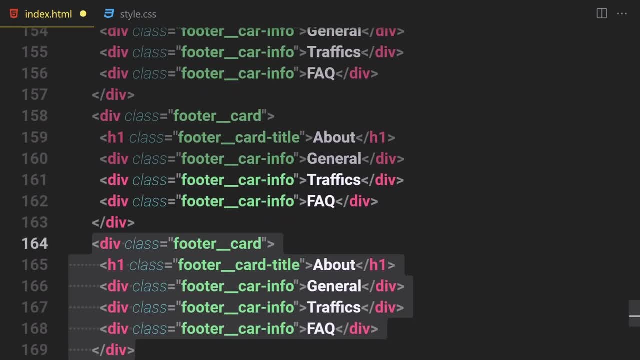 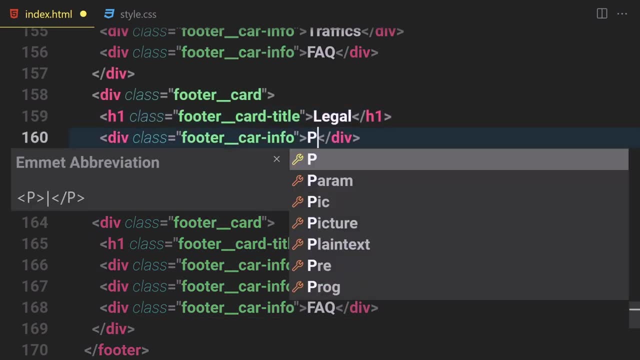 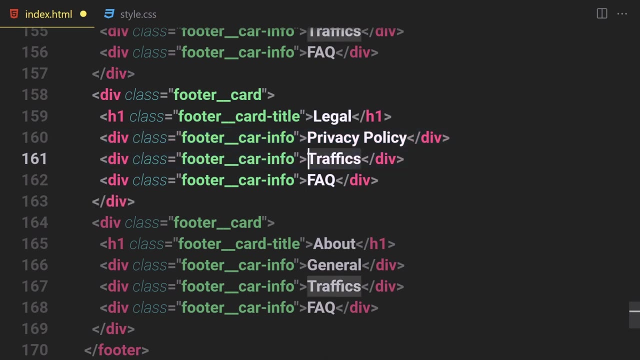 have to do. we are going to be duplicating that one and two. so we are going to be duplicating that two times as a title. i'm going to change that to like legal. and then we have a privacy and policy. yes, p-r-i-v-s-c-y and p-o-l-i-c-y. so privacy and policy. so terms uh of uses, u-s-e-s lowercase. 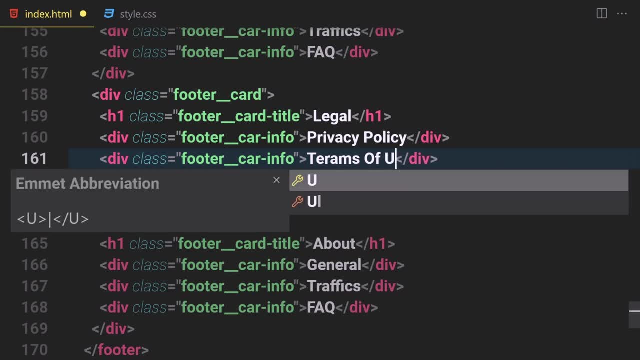 u-s-e-s. oh, my goodness, i guess something went wrong in my shift key, so use this. uh, all right, so then, finally, we are going to be writing a pam me mints, okay, so underneath all of them. now let's just change the title to be a contact and also. 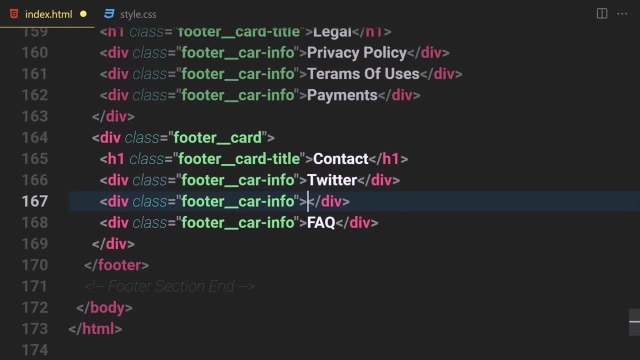 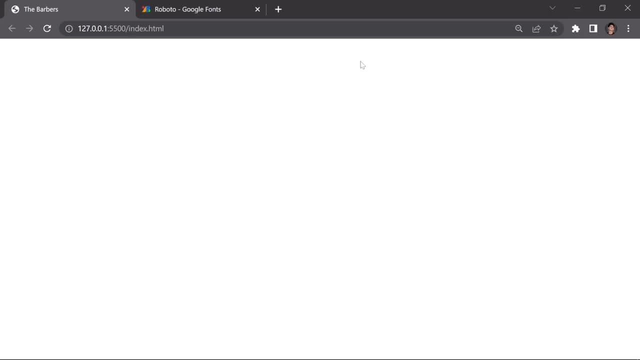 this journal will be now set to twitter and also this is going to be instagram. if you want to follow me on this, let's just write that to facebook. so if you save that, and oh my goodness, and this word photo right here. so now let's just get into the style sheet. and now let's just style. 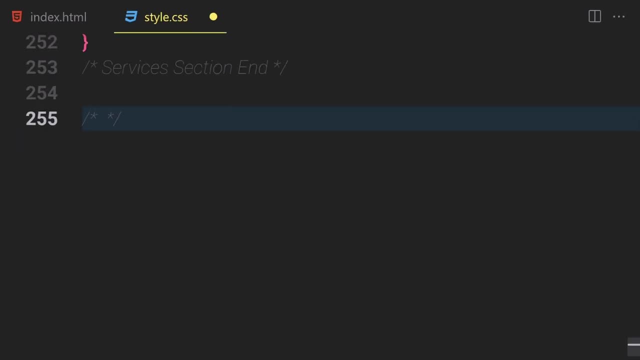 that a bit. so first of all, let me just write a comment for myself. uh, folder section: start and do a comment for myself. uh, photo section: start and do a comment for myself. uh, photo section: start and do click at that and this is going to be the end of that further section. so what do we have to do? we click at that and this is going to be the end of that further section. so what do we have to do? we click at that and this is going to be the end of that further section. so what do we have to do? we are going to be, first of all, selecting. 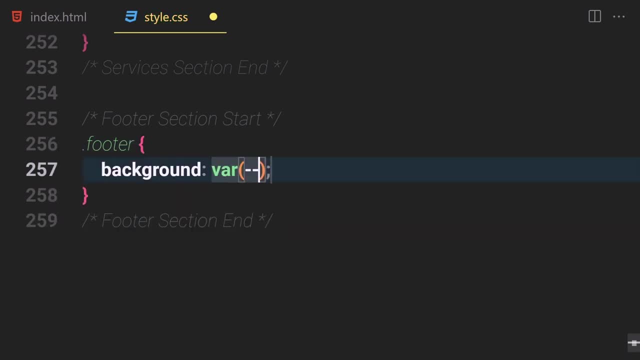 are going to be first of all selecting, are going to be first of all selecting our folder. and now let's just change the our folder. and now let's just change the our folder, and now let's just change the background color to be like one of their. 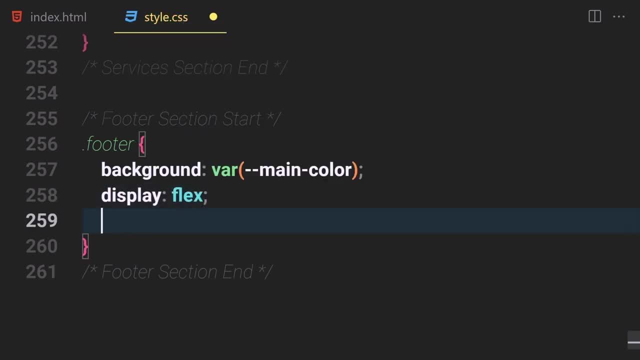 background color to be like one of their background color, to be like one of their main color, which we already choose and main color which we already choose and main color which we already choose, and display will be now set to totally flex. display will be now set to totally flex. 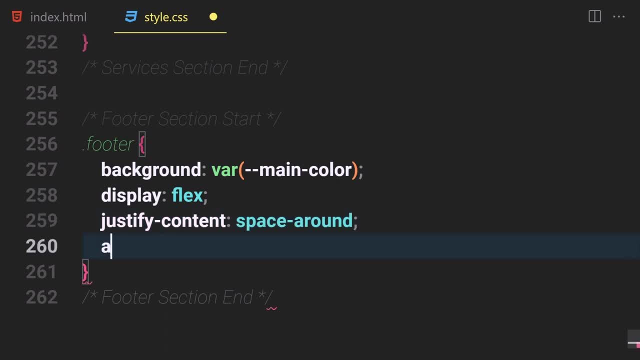 display will be now set to totally flex. justify counter will be now set to space. justify counter will be now set to space. justify counter will be now set to space around, because we want everything to be around, because we want everything to be around, because we want everything to be uh, i mean like we want a little bit of. 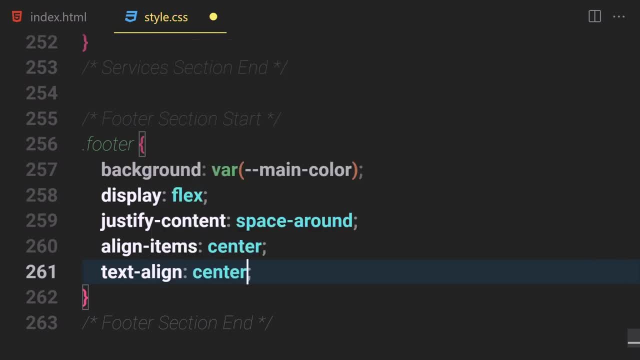 uh, i mean like we want a little bit of. uh, i mean like we want a little bit of spacing in there and text alignment will spacing in there and text alignment will spacing in there and text alignment will be also set to center. be also set to center. 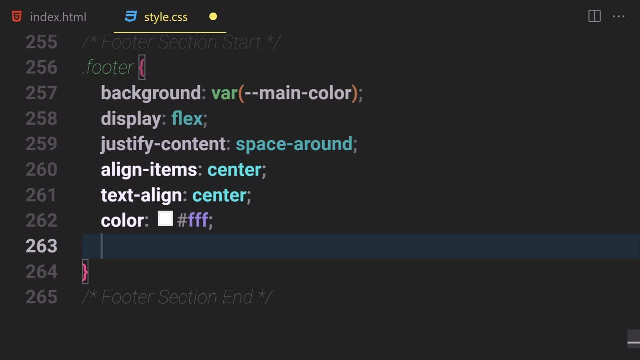 be also set to center. okay, so what else do we have to do? we, okay. so what else do we have to do? we okay, so what else do we have to do? we want the color to be totally pure white. want the color to be totally pure white. 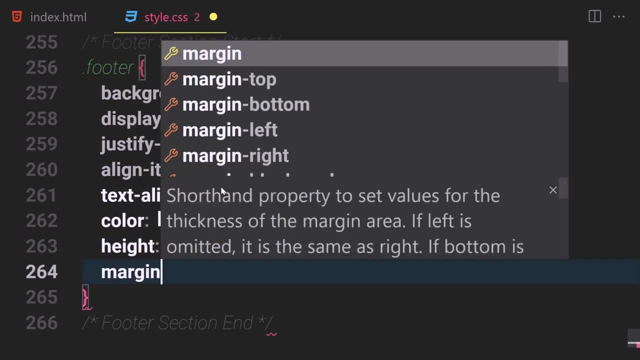 want the color to be totally pure white and height will be now set to five or 50 and height will be now set to 50 and height will be now set to 50 vh margin top. i'm gonna give him like 10 vh margin top. i'm gonna give him like 10. 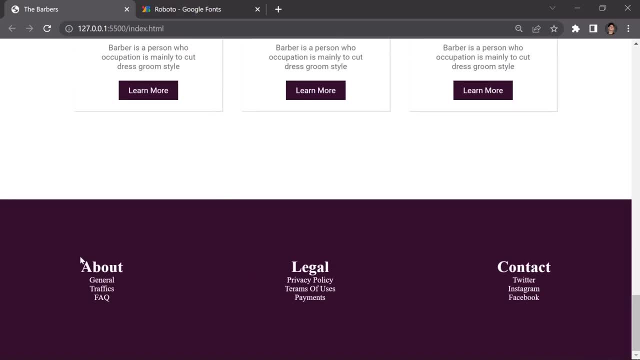 vh margin top. i'm gonna give him like 10 rooms. so if you sell that rooms, so if you sell that rooms, so if you sell that- and this is how it looks like for now i. and this is how it looks like for now i. and this is how it looks like for now. i know it's ugly. now let's just tile that. 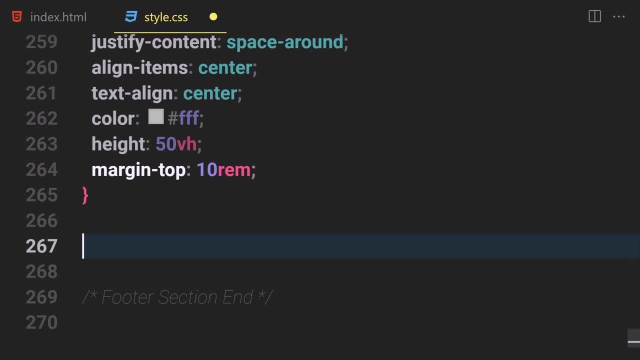 know it's ugly now, let's just tile that. know it's ugly now, let's just tile that. titles and stuff, so titles and stuff, so titles and stuff. so, first of all, we have to select that um. first of all, we have to select that um. first of all, we have to select that um. what do we call it footer? dash, dash. 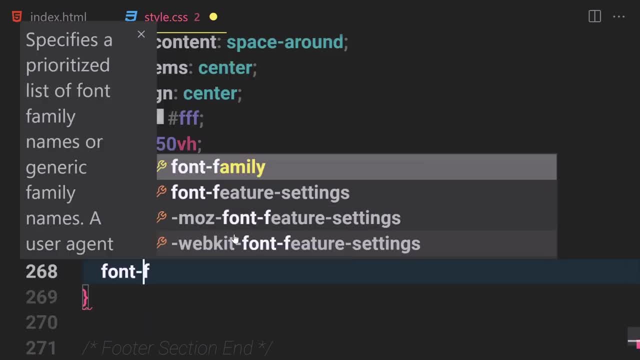 what do we call it footer dash dash? what do we call it footer dash dash card and then dash title: okay, so inside card, and then dash title. okay, so inside card, and then dash title. okay, so inside there. we are going to be just changing there. we are going to be just changing. 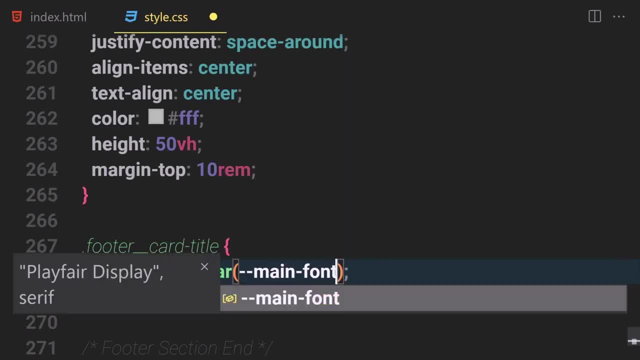 there, we are going to be just changing the font family to like a main font, not the font family. to like a main font, not the font family. to like a main font, not main color but main font. okay, so main color, but main font. okay. so main color, but main font. okay. so underneath that we are going to be using 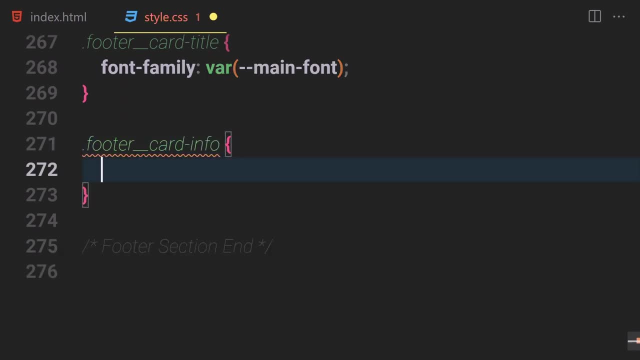 underneath that we are going to be using, underneath that we are going to be using footer dash card and then dash what info- footer dash card. and then dash what info- footer dash card and then dash what info? let's just select there and we are going. let's just select there and we are going. 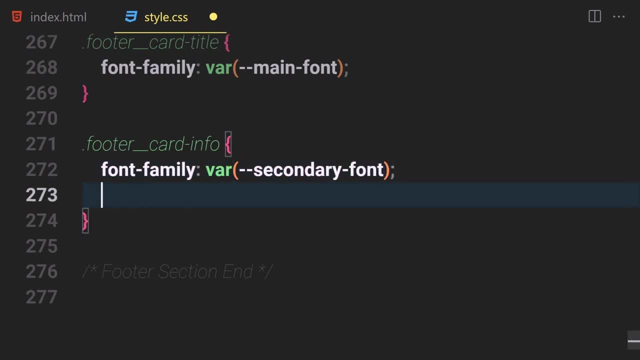 let's just select there- and we are going to be changing the font family- to like to be changing the font family, to like to be changing the font family to like part secondary font and also the line part secondary font and also the line part secondary font and also the line height will be now set to two rims. so if 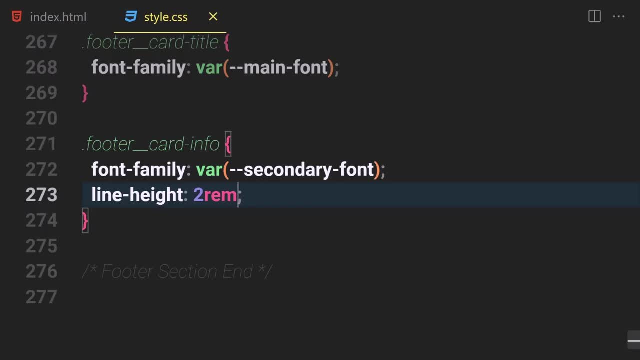 height will be now set to two rims. so if height will be now set to two rims, so if you sell that, you sell that, you sell that, and this is how it looks like right now. and this is how it looks like right now. and this is how it looks like right now. so i guess we messed it up something. so 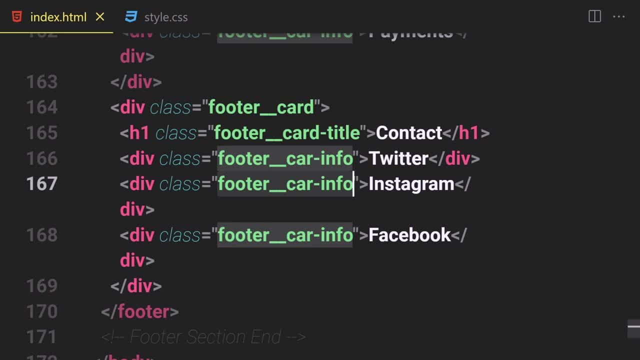 so i guess we messed it up something. so so i guess we messed it up something. so we have folder card info. we have folder card info. we have folder card info. copy that in here, copy that in here, copy that in here, and i want to paste it right here i. 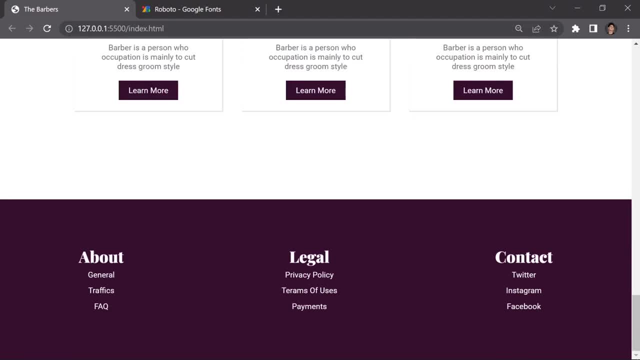 and i want to paste it right here. i and i want to paste it right here. i guess both of them was fine. guess both of them was fine. guess both of them was fine anyway. so now we get that, i guess some anyway. so now we get that, i guess some. 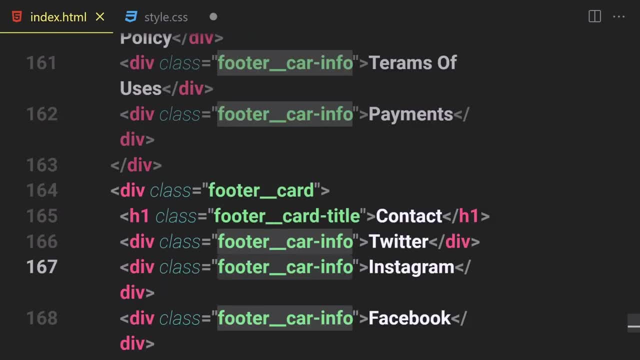 anyway. so now we get that, i guess some card, card, card. we have to put a card in there. so this is, we have to put a card in there. so this is, we have to put a card in there. so this is going to be the d going to be the d. 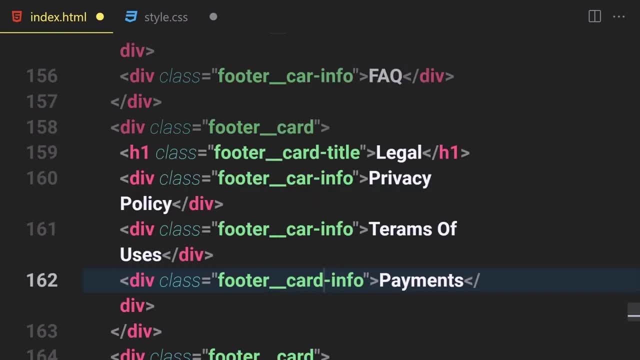 going to be the d, d and d. this is part of these for them. d and d. this is part of these for them. d and d. this is part of these for them. my apologies, my apologies, my apologies. and d and d, so save that. and d and d, so save that. 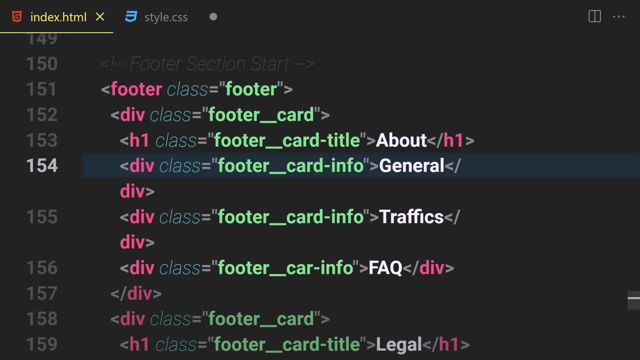 and d and d. so save that. and this is how it looks like phone i. and this is how it looks like phone i and this is how it looks like phone i guess, guess, guess. uh, something is wrong card and also. uh, something is wrong card and also. 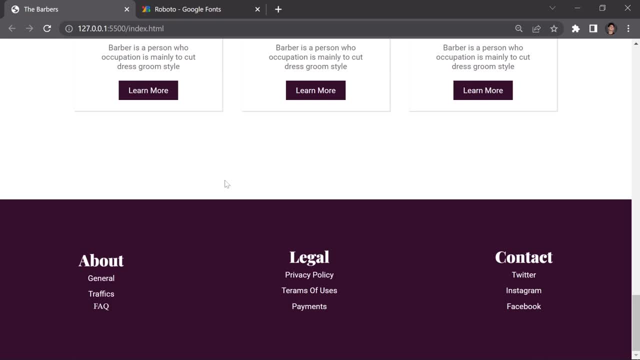 uh, something is wrong. card and also save this file. save this file. save this file. all right, so now it's looking better. all right, so now it's looking better. all right, so now it's looking better. so now we are totally done with our. so now we are totally done with our. 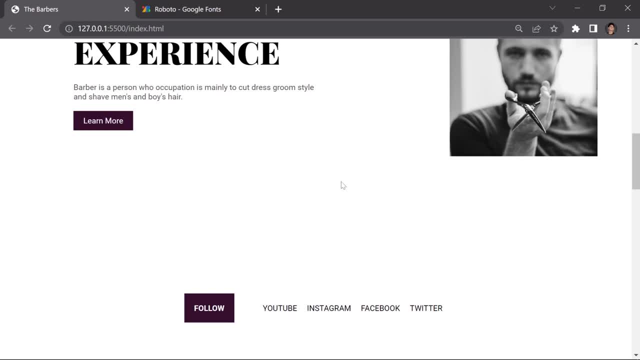 so now we are totally done with our project. but the final thing which you project, but the final thing which you project, but the final thing which you have to do is that we have to write a have to do is that we have to write a have to do is that we have to write a media queries to make the site totally. 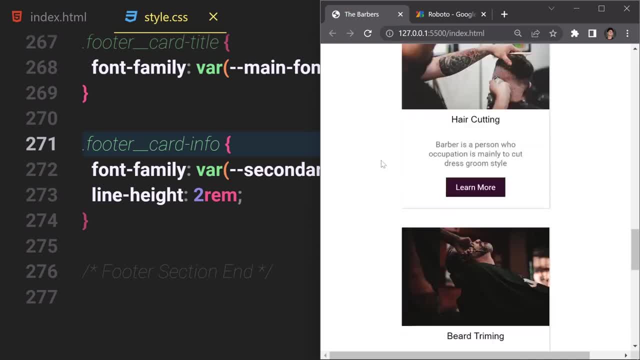 media queries to make the site totally. media queries to make the site totally responsive. so i'm going to just make responsive. so i'm going to just make responsive. so i'm going to just make that to smaller screen size and you can that to smaller screen size and you can. 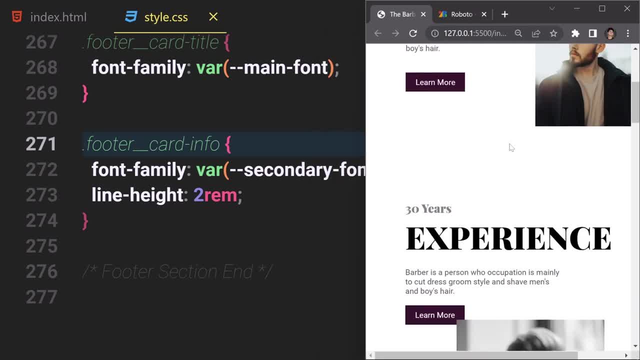 that to smaller screen size and you can see that it's not that much horrible. but see that it's not that much horrible, but see that it's not that much horrible. but if you just go a little bit more smaller, if you just go a little bit more smaller, 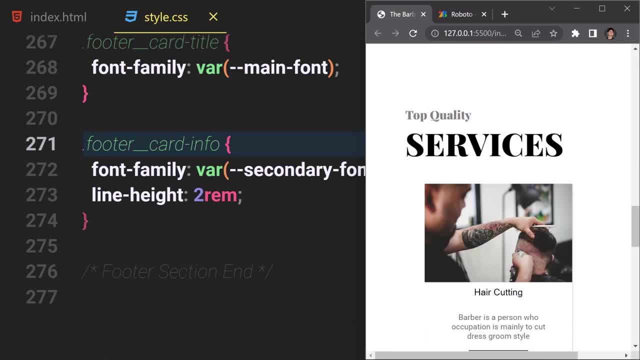 if you just go a little bit more smaller. so everything, just so, everything, just so everything just looking a bit awful. so for that we have looking a bit awful, so for that we have looking a bit awful, so for that we have to write a media queries. to write a media queries. 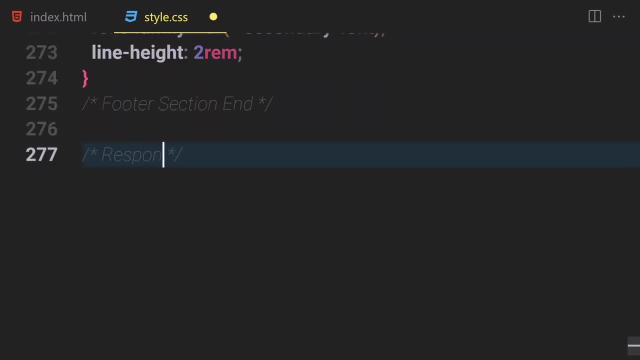 to write a media queries. so i'm going to just write finally the. so i'm going to just write finally the. so i'm going to just write finally the responsiveness. i guess that's the responsiveness. i guess that's the responsiveness, i guess that's the spelling, i'm not sure. but first of all, 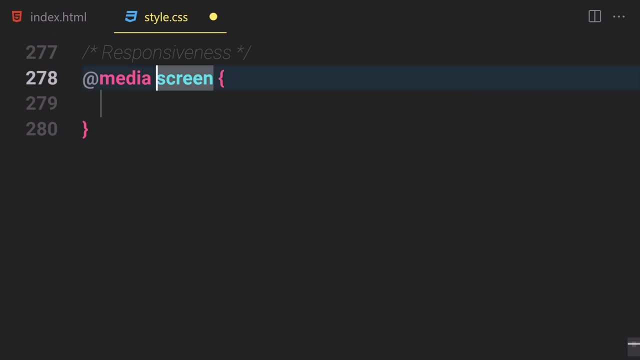 spelling: i'm not sure, but first of all, spelling: i'm not sure, but first of all, let's just write: add symbol and media. let's just write: add symbol and media. let's just write: add symbol and media. or only screen and what, and or only screen and what and. 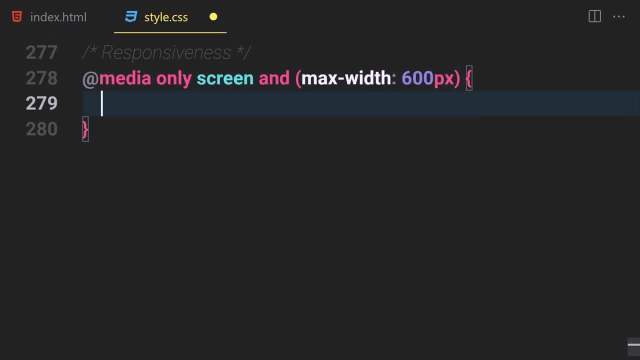 or only screen and what? and max width, if the media query max width, max width. if the media query max width, max width. if the media query max width is like 600 pixel. so if you want to is like 600 pixel. so if you want to is like 600 pixel. so if you want to select your header dash content, first of. 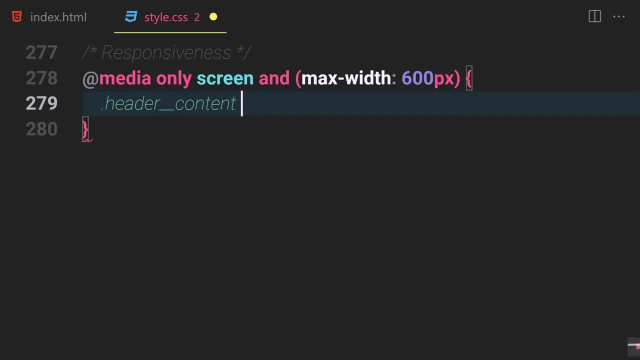 select your header dash content. first of select your header dash content, first of all, the header content. so what do you all the header content? so what do you all the header content? so what do you want to do with that, want to do with that, want to do with that? i'm going to select that and align items. 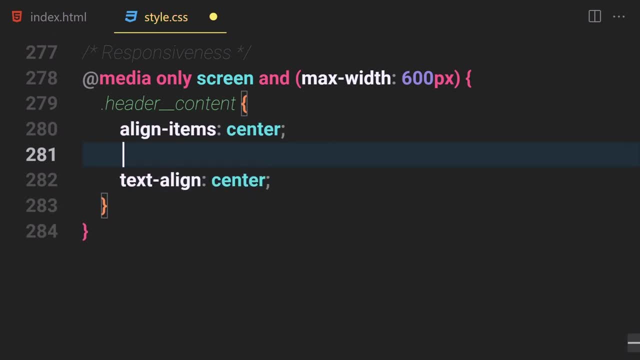 i'm going to select that and align items. i'm going to select that and align items. i'm going to set that to center and text. i'm going to set that to center and text. i'm going to set that to center and text alignment. i'm going to also set that to. 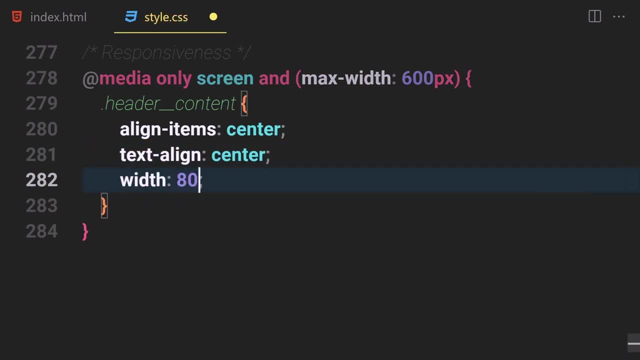 alignment: i'm going to also set that to alignment. i'm going to also set that to center. okay, so the width, i'm going to center. okay, so the width, i'm going to center. okay, so the width, i'm going to give them like 70, give them like 70. 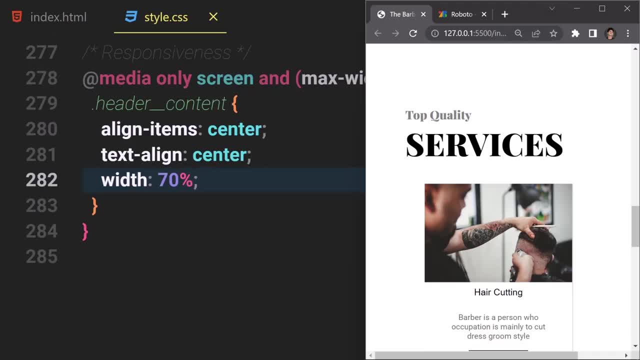 give them like 70, uh percent in this case. so i'm going to uh percent in this case. so i'm going to uh percent in this case. so i'm going to write 70 and if you sell that, write 70. and if you sell that, 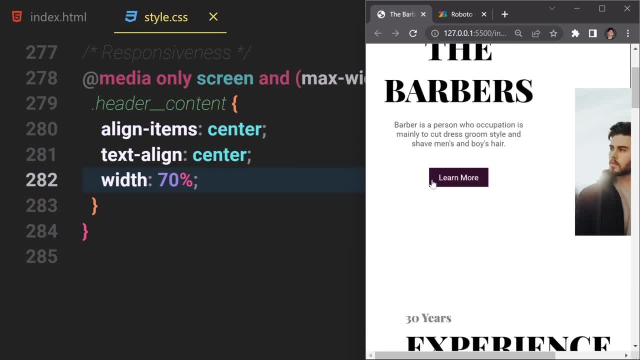 write 70, and if you sell that, and this is how it looks like you know, and this is how it looks like you know, and this is how it looks like you know what, let me just show you what. let me just show you what. let me just show you: uh, okay, something isn't working, so hdr. 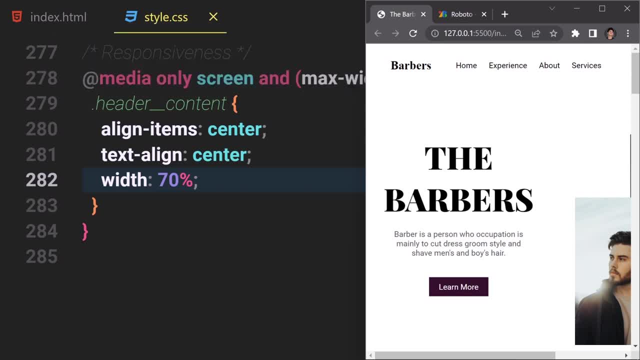 uh okay, something isn't working, so hdr. uh okay, something isn't working, so hdr. header content, header content. header content. so nt nt x line is center, so nt nt x line is center, so nt nt x line is center. uh, you know what i'm going to also take. uh, you know what i'm going to also take, uh, you know what i'm going to also take: care of these images so that they look a care of these images, so that they look a care of these images, so that they look a bit better, bit better. 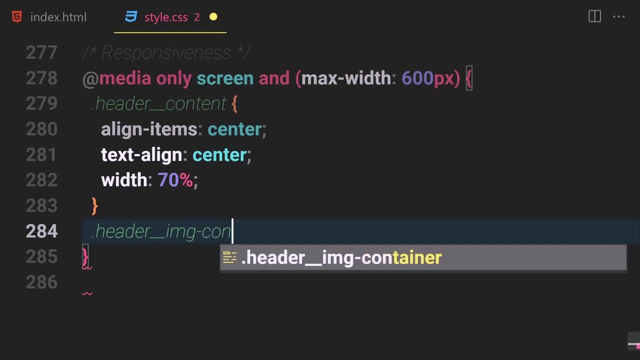 bit better. i'm going to select my header dash dash. i'm going to select my header dash dash. i'm going to select my header dash dash image and then container like so and image and then container like so and image and then container like so, and just write a display of none towards so. just write a display of none towards. so just write a display of none towards. so we are going to be also removing that. we are going to be also removing that. we are going to be also removing that. and this is how it looks like for now. and this is how it looks like for now. 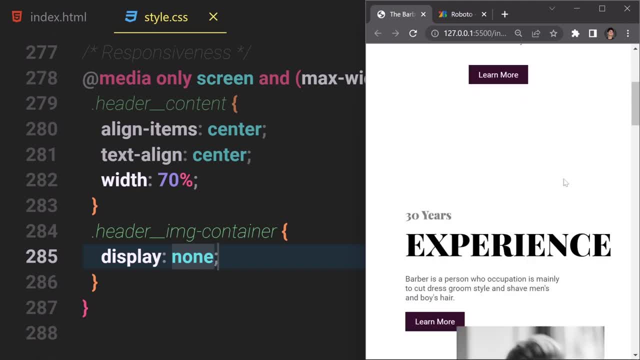 and this is how it looks like for now. okay, so everything is perfectly centered. okay, so, everything is perfectly centered. okay, so everything is perfectly centered, and that's done. now let's just take care, and that's done. now let's just take care, and that's done. now let's just take care of these sections like: 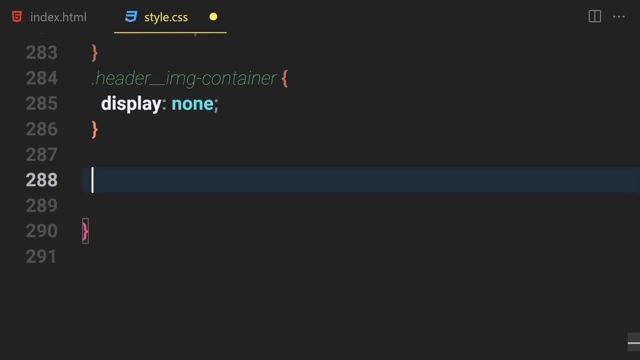 of these sections, like, of these sections like: uh, what do we call experience sections? uh, what do we call experience sections? uh, what do we call experience sections? so, first of all, we are going to be so, first of all, we are going to be so, first of all, we are going to be writing xp experience right here, and 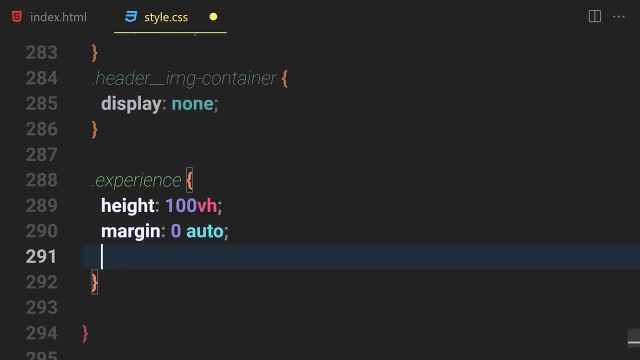 writing xp experience right here and writing xp experience right here. and height: i'm going to give him like 100 vh height. i'm going to give him like 100 vh height. i'm going to give him like 100 vh and margin would be zero. auto, so that. 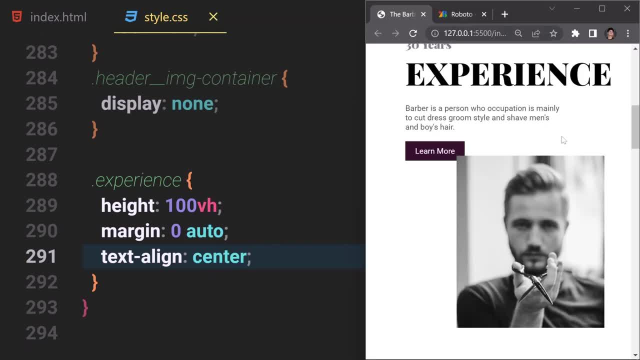 and margin would be zero auto. so that, and margin would be zero auto, so that everything is now totally at the center. everything is now totally at the center. everything is now totally at the center. so save that, so, save that, so save that. and this is how it looks like right now. 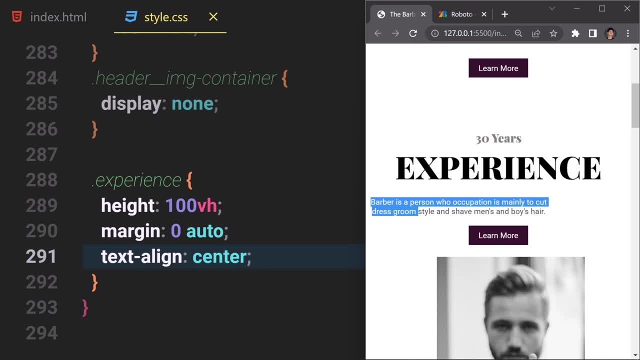 and this is how it looks like right now. and this is how it looks like right now. okay, so i guess we must have something. okay, so i guess we must have something. okay, so i guess we must have something in here which is um twitter, in here which is um twitter. 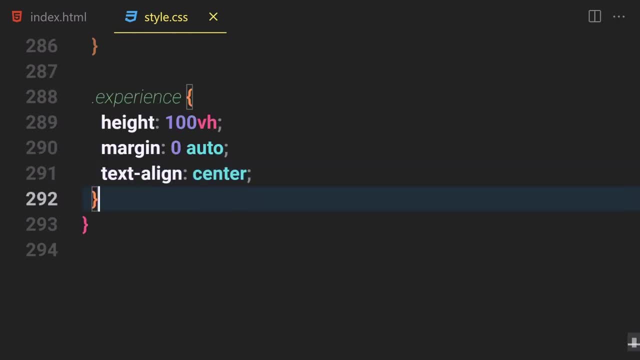 in here, which is um twitter, which is experience heading, i guess. so which is experience heading, i guess. so which is experience heading, i guess. so let's just select there real quick, let's just select there real quick. let's just select there real quick: um experience, um experience. 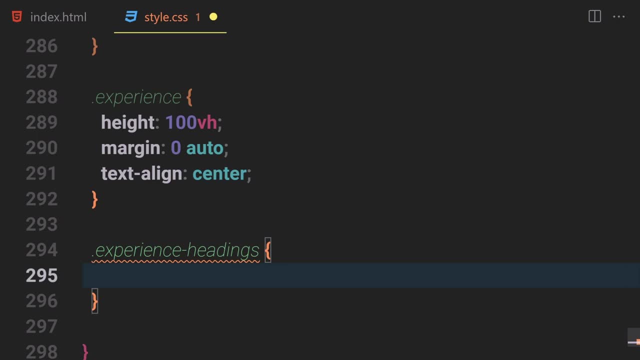 um experience. and now let's just select our headings. and now let's just select our headings. and now let's just select our headings. experience headings. i'm going to just experience headings. i'm going to just experience headings. i'm going to just increase the sizing of font size to be. 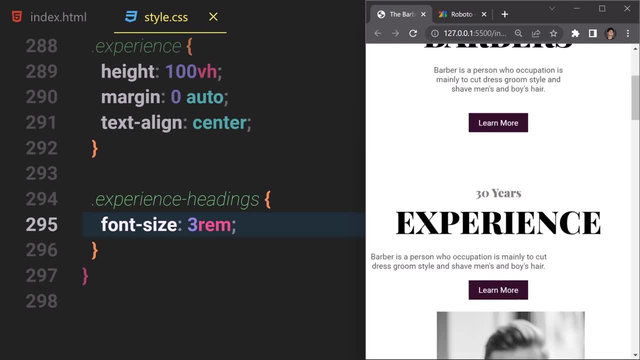 increase the sizing of font size to be. increase the sizing of font size to be like three ram. and if you sell that like three ram, and if you sell that like three ram, and if you sell that, uh okay, something isn't working the way. uh okay, something isn't working the way. 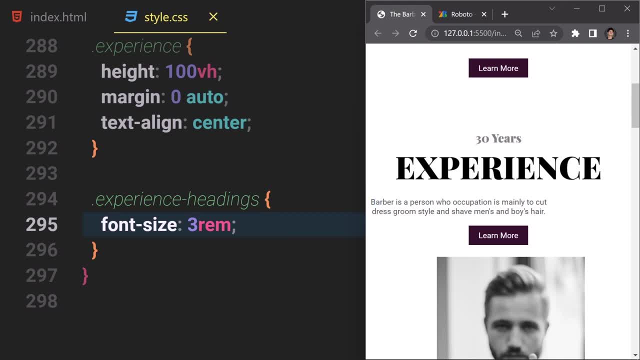 uh, okay, something isn't working the way. we expect them to work, so we expect them to work, so we expect them to work. so what is it when this call class card? so what is it when this call class card? so what is it when this call class card? so we gotta go to. 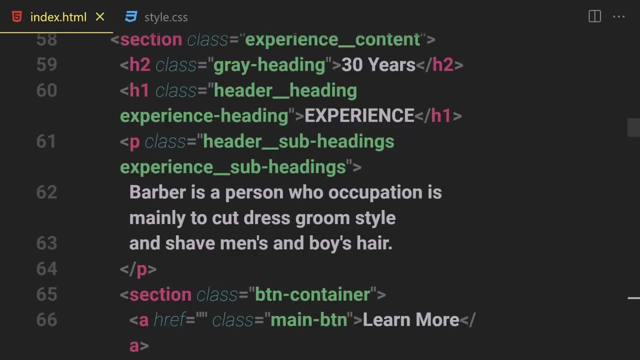 we gotta go to. we gotta go to uh experience section, and then we have uh experience section, and then we have uh experience section, and then we have our, our, our subheadings, i guess so subheadings, i guess so subheadings, i guess so there's some headings, or you know what. 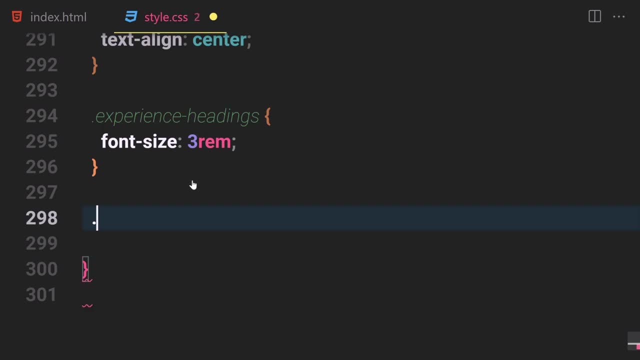 there's some headings, or you know what? there's some headings, or you know what? experience experience experience- subheadings- i'm going to select that subheadings. i'm going to select that subheadings. i'm going to select that. and what else can we do with that? i'm 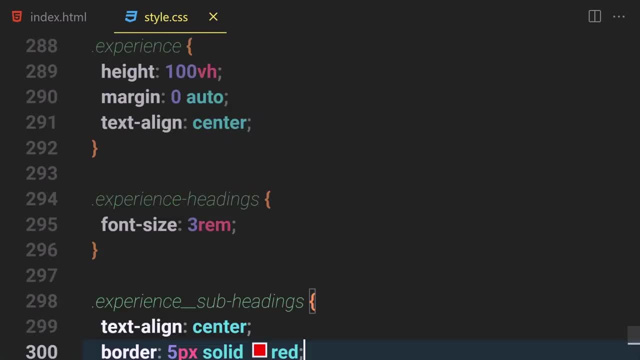 and what else can we do with that? i'm and what else can we do with that? i'm red, and if you sell that red, and if you sell that red, and if you sell that, all right, so that's that, what can we do? all right, so that's that, what can we do? 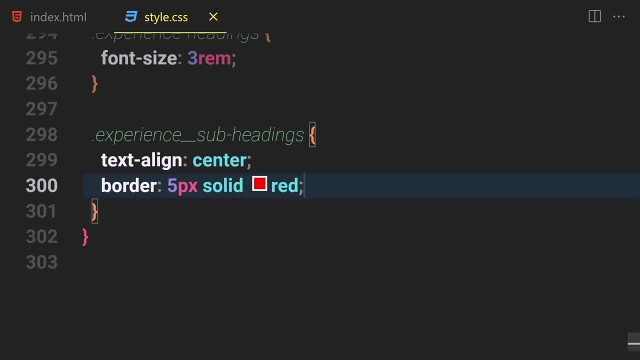 all right. so that's that. what can we do with uh, with uh, with uh? margin zero auto. so what else does that margin zero auto? so what else does that margin zero auto? so what else does that want from us? want from us, want from us? if you just heard margin zero auto in 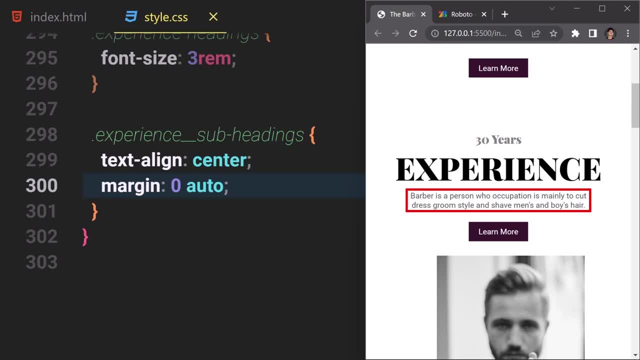 if you just heard margin zero auto in, if you just heard margin zero auto in this case, this case, this case. all right, that's looking better. all right, that's looking better. all right, that's looking better. yep, that's looking better. yep, that's looking better. 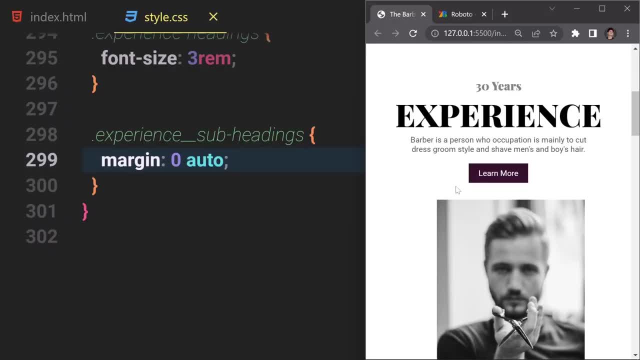 yep, that's looking better anyway. so you can provide margins in anyway. so you can provide margins in anyway. so you can provide margins in there if you want to. so if you just there if you want to. so if you just there if you want to. so if you just remove that text alignment. 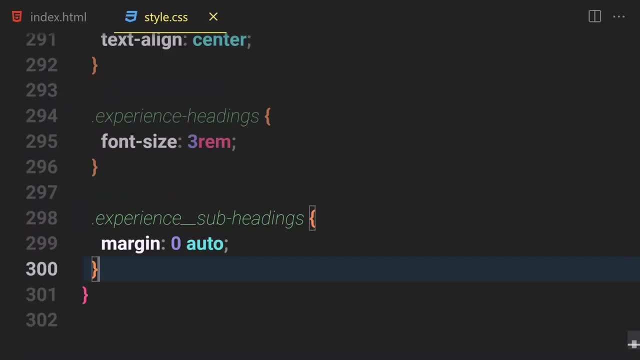 remove that text alignment. remove that text alignment. it's still working, and yeah, that's cool, it's still working and yeah, that's cool, it's still working and yeah, that's cool. now, what else do we have to do now? what else do we have to do? 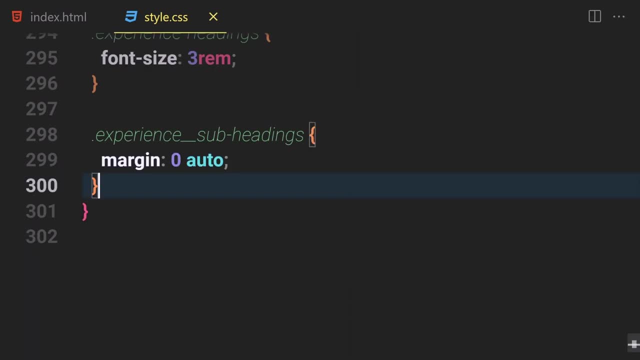 now, what else do we have to do? let's select that image. let's select that image. let's select that image, and. or you know what that's fine, but, and, or you know what that's fine but, and, or you know what that's fine, but you know what i'm going to select it. 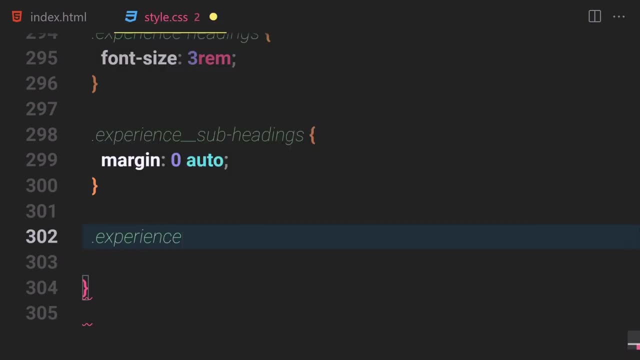 you know what i'm going to select it. you know what i'm going to select it and change the size of it. so experience and change the size of it. so experience and change the size of it. so experience. uh, what experience, img. so now let's just 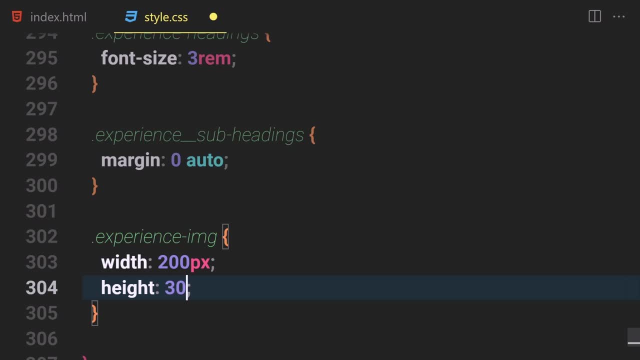 uh, what experience img. so now let's just: uh, what experience img. so now let's just select that, and the width will be 200. select that, and the width will be 200. select that and the width will be 200 pixel. the height will be just 300 pixels. 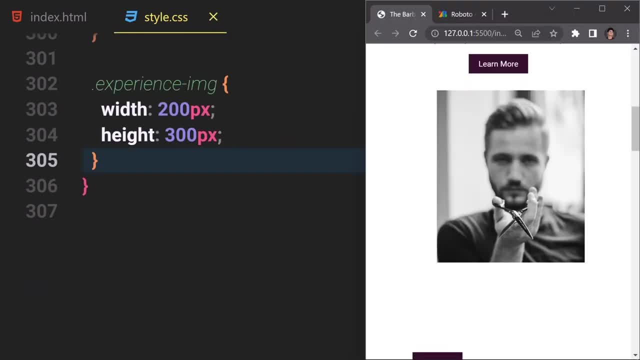 pixel: the height will be just 300 pixels. pixel: the height will be just 300 pixels. okay, so now let's just provide. okay, so now let's just provide. okay, so now let's just provide. uh, i guess that would be fine, so if you. uh, i guess that would be fine, so if you. 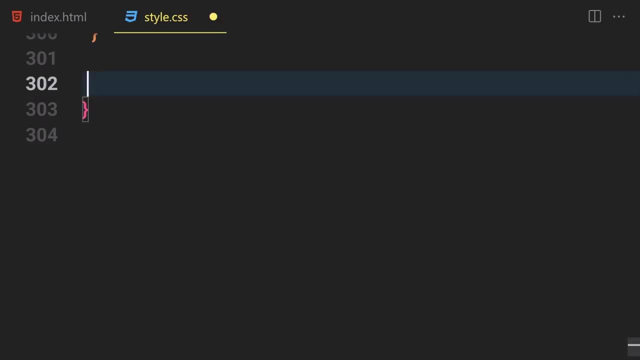 uh, i guess that would be fine. so if you save that you know what that's looking, save that, you know what that's looking. save that. you know what that's looking- awful. so i'm going to remove this awful. so i'm going to remove this awful. so i'm going to remove this experience image section from there and 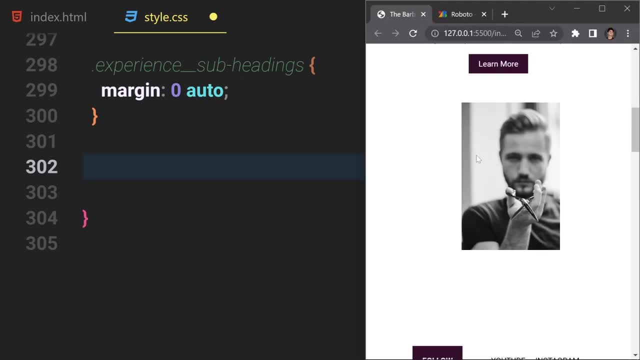 experience image section from there and experience image section from there, and let's just work with that. let's just work with that. let's just work with that. subheadings, um, subheadings, um, subheadings, um. now, let's just work with these buttons. now, let's just work with these buttons. 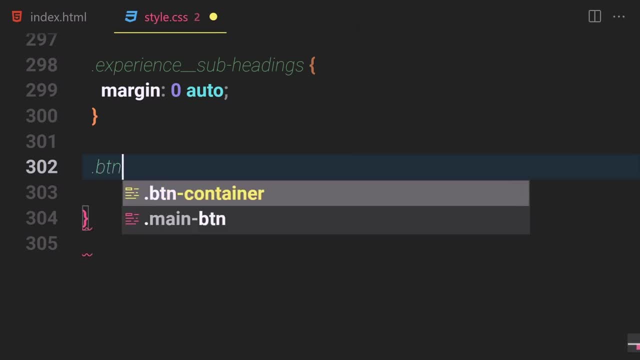 now let's just work with these buttons and stuff like these, so, and stuff like these, so and stuff like these. so, first of all, i'm going to just write. first of all, i'm going to just write. first of all, i'm going to just write like a buttons container, let's just 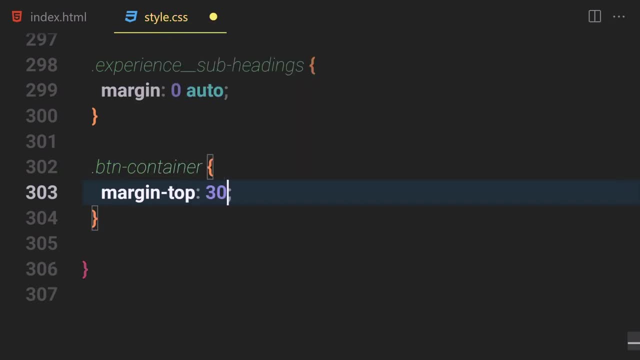 like a buttons container. let's just like a buttons container. let's just select that and i'm going to use a select that, and i'm going to use a select that and i'm going to use a margin top for all of these um. margin top for all of these um. 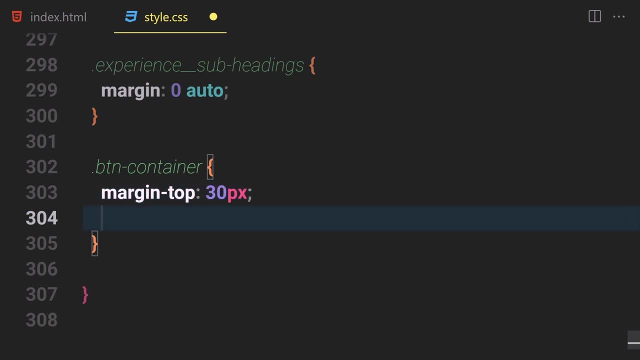 margin top for all of these: um buns container and i'm going to provide a buns container and i'm going to provide a buns container and i'm going to provide a margin margin top of 30 pixel. margin margin top of 30 pixel. 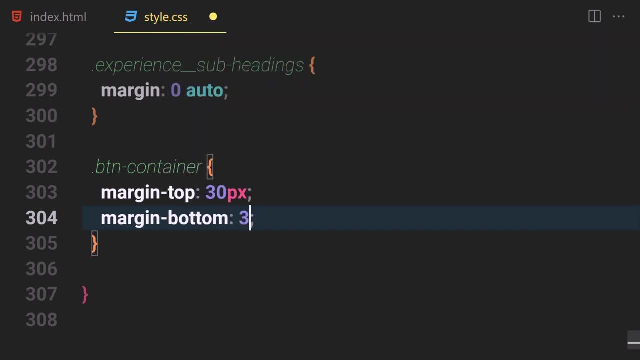 margin margin top of 30 pixel top and i'm going to also provide a top and i'm going to also provide a top and i'm going to also provide a margin for the bottom like 3.5 rems. so margin for the bottom like 3.5 rems. so 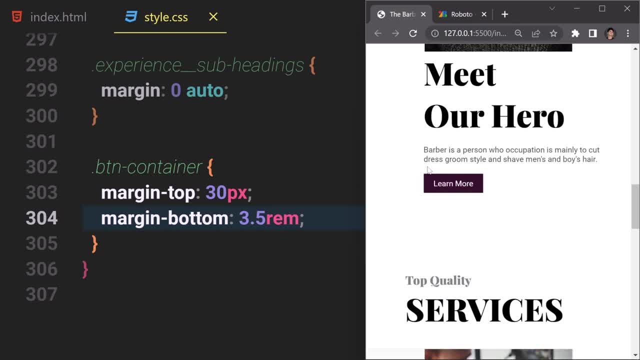 margin for the bottom, like 3.5 rems. so if you sell that, if you sell that, if you sell that, and i guess that's looking better right, and i guess that's looking better right, and i guess that's looking better right now. okay, now, okay. 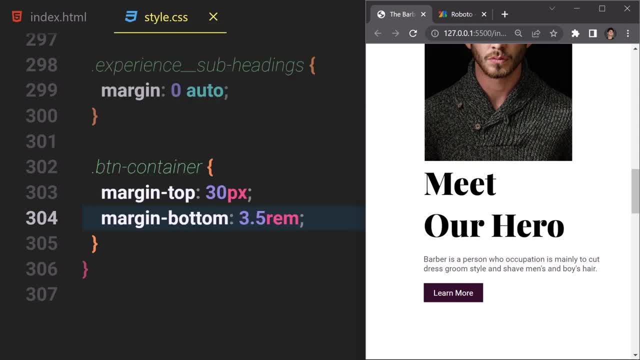 now okay. so if you want to change it more, you can. so if you want to change it more, you can. so if you want to change it more, you can also change that. if you want to also change that, if you want to also change that, if you want to, and now let's just style, or you know. 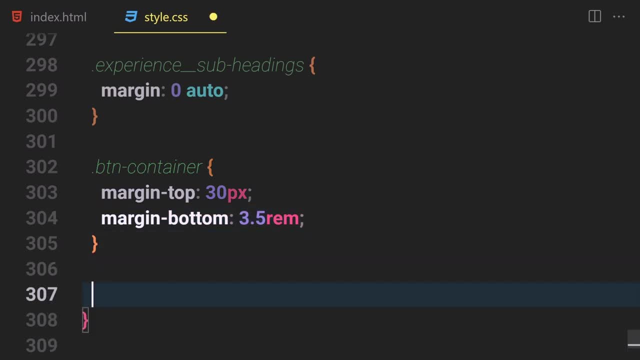 and now let's just style, or you know, and now let's just style, or you know what. let's just remove this, what. let's just remove this, what? let's just remove this follow button because it's looking awful. follow button because it's looking awful. follow button because it's looking awful. so i'm gonna write like a follow. 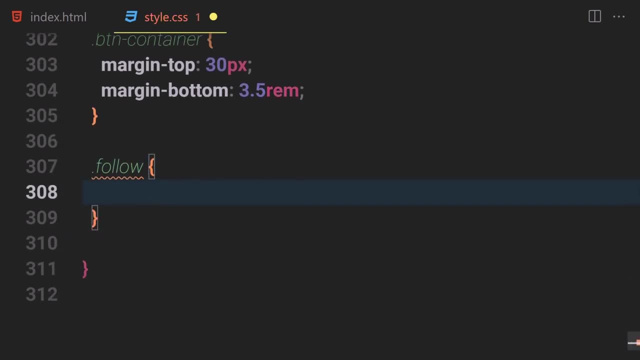 so i'm gonna write like a follow. so i'm gonna write like a follow in here, and if you want to leave it in here, and if you want to leave it in here and if you want to leave it there, so you can also just tweak around. 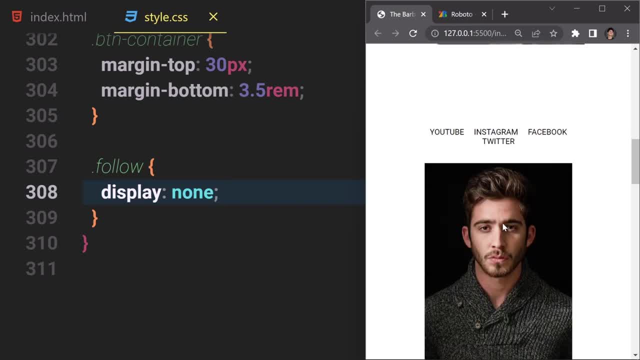 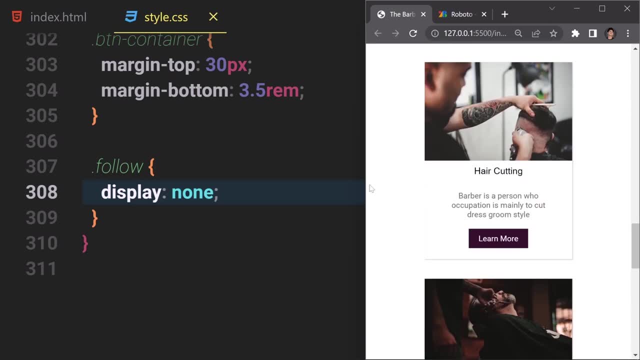 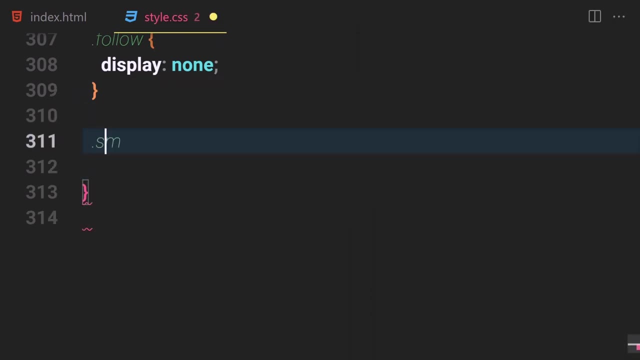 there, so you can also just tweak around there, so you can also just tweak around the things, but i'm going to just remove the things. but i'm going to just remove the things, but i'm going to just remove that sm container or what sm container, that sm container or what sm container. 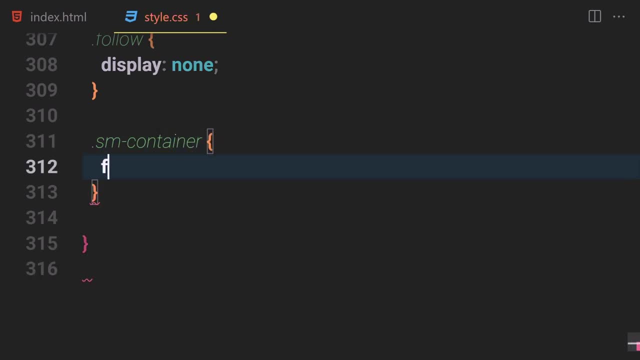 that sm container or what sm container? let's just select that. and what do we? let's just select that. and what do we? let's just select that. and what do we have to do with that? so we are going to have to do with that. so we are going to. 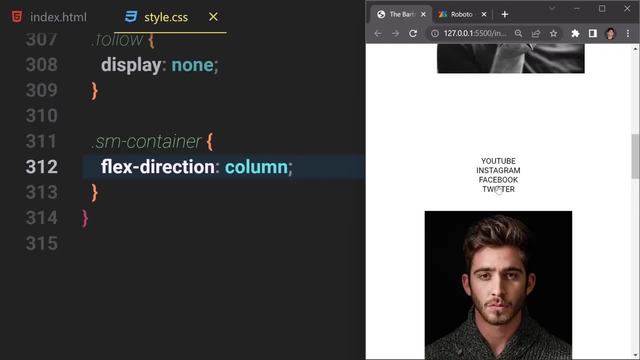 have to do with that. so we are going to just using a flex direction of columns, just using a flex direction of columns, just using a flex direction of columns if you save that, and yeah, that's looking. if you save that and yeah, that's looking. if you save that and yeah, that's looking better. 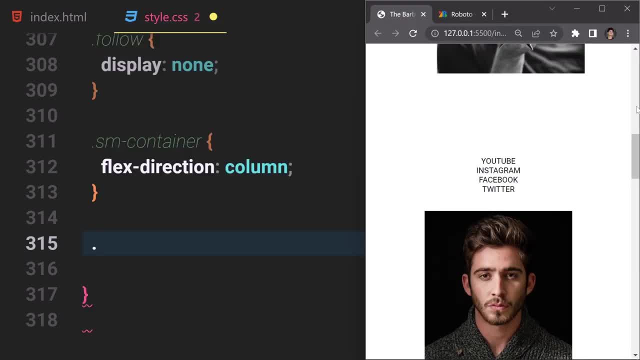 better, better anyways. so now let's just select our anyways. so now let's just select our anyways. so now let's just select our list items. so where is our list item and list items? so where is our list item and list items? so where is our list item? and here here is. so now let's just pour a. 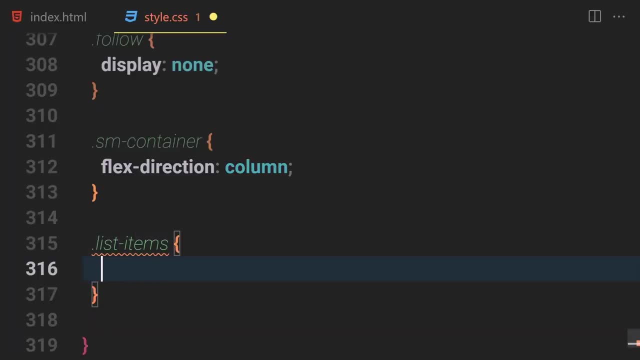 here. here is. so now let's just pour a here. here is. so now let's just pour a little bit of spacing in there. so i'm little bit of spacing in there. so i'm little bit of spacing in there. so i'm going to just write, like a list items. going to just write like a list items. going to just write like a list items and margin. i'm going to give like 10 and margin. i'm going to give like 10 and margin. i'm going to give like 10 pixel all around, pixel, all around. 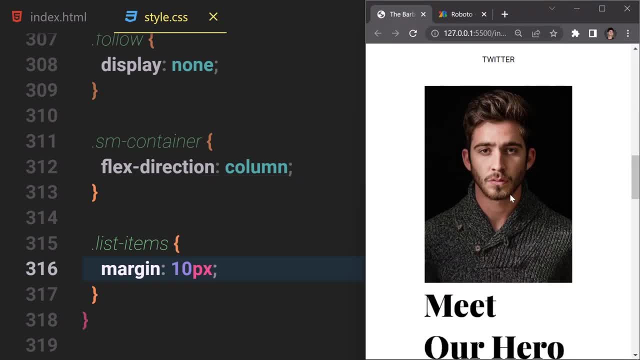 pixel all around, and i guess that's looking better if, and i guess that's looking better if, and i guess that's looking better if you want to change it on other ways. so you want to change it on other ways, so you want to change it on other ways, so you can totally do that if you want to. 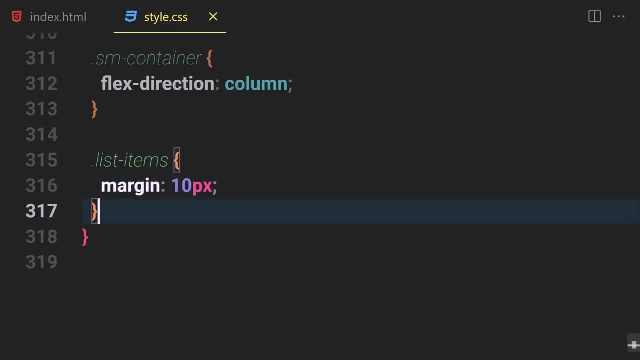 you can totally do that if you want to. you can totally do that if you want to, but in my case that's looking totally, but in my case that's looking totally, but in my case that's looking totally, okay, okay, okay. and hero image container. so let's just 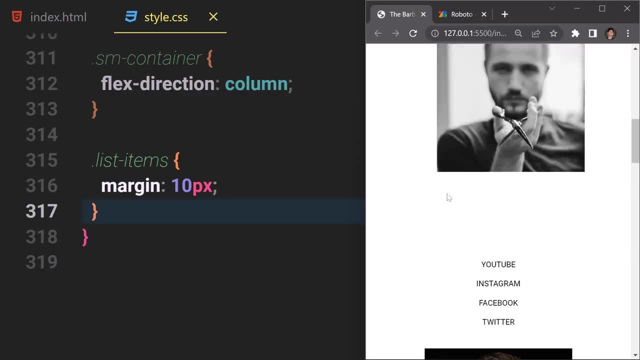 and hero image container. so let's just and hero image container. so let's just work on this hero image container. work on this hero image container. work on this hero image container, like so. so i'm going to just select that. like so. so i'm going to just select that. 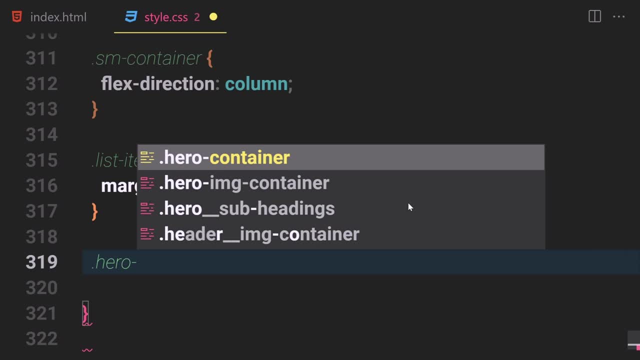 like so. so i'm going to just select that first of all, first of all, first of all: uh, we have our hero, then image. uh, we have our hero, then image. uh, we have our hero, then image: uh, iron, so we have image, and then, uh, iron, so we have image, and then uh, iron. so we have image and then container. so what do we have to do? i'm container, so what do we have to do? i'm container, so what do we have to do? i'm going to just give you know what that's. going to just give you know what that's. going to just give you know what that's looking for. that's looking fine. i'm not looking for. that's looking fine. i'm not looking for. that's looking fine. i'm not going to work with that uh hero image. going to work with that uh hero image. 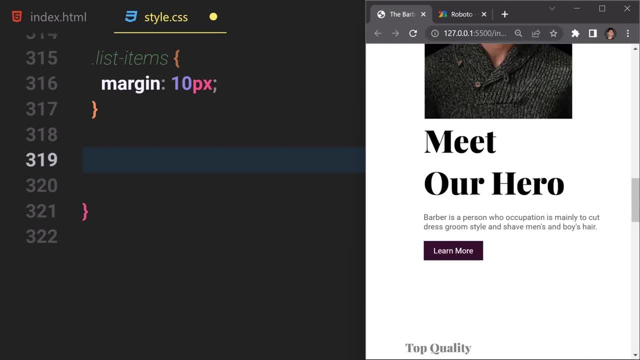 going to work with that uh hero image container, because this is looking totally container. because this is looking totally container, because this is looking totally okay. if you want to change that, so you okay. if you want to change that, so you okay. if you want to change that, so you can totally do that if you want to. but 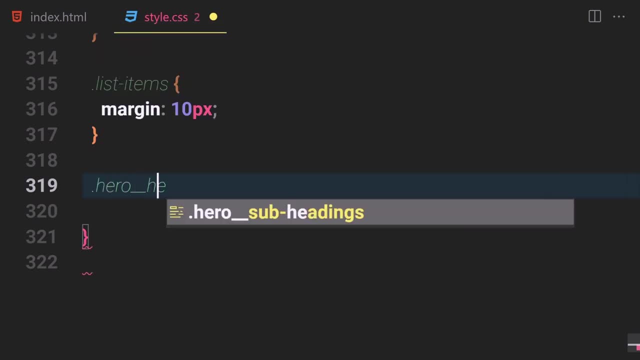 can totally do that if you want to. but can totally do that if you want to, but in my case it's looking better, and then in my case it's looking better, and then in my case it's looking better, and then we have a hero. um what? 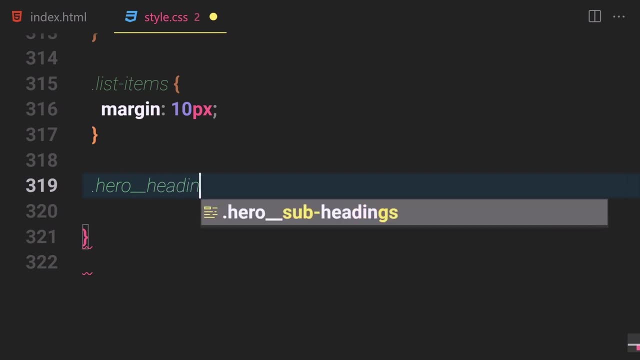 we have a hero, um what? we have a hero um what? hero headings, not some headings. but we hero headings, not some headings, but we hero headings, not some headings. but we have a hero, have a hero, have a hero headings. so we are going to be just writing. 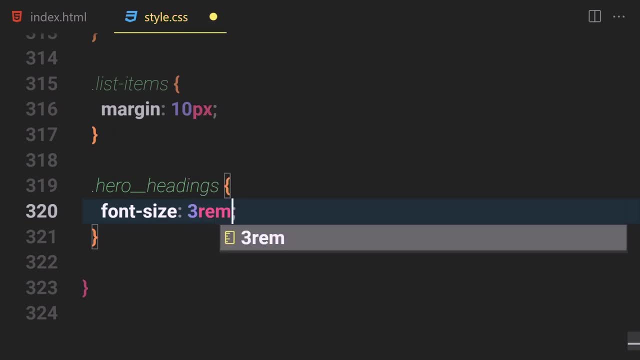 headings. so we are going to be just writing headings, so we are going to be just writing a font size, a font size, a font size of three rims, so if you sell that, and of three rims, so if you sell that, and of three rims, so if you sell that. and this is a little bit smaller than usual. 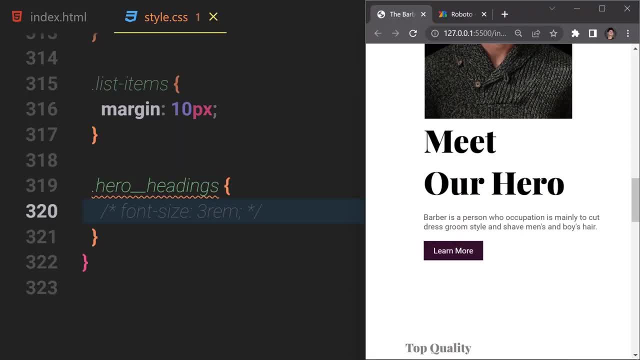 this is a little bit smaller than usual. this is a little bit smaller than usual, so i guess that's looking better. if you so, i guess that's looking better. if you so, i guess that's looking better. if you want to leave it the way it is, so you. 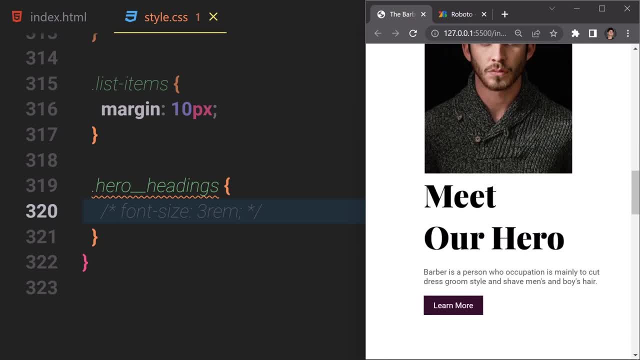 want to leave it the way it is, so you want to leave it the way it is, so you can just uncomment it. and this is how can just uncomment it. and this is how can just uncomment it, and this is how it will look like, if you want to. 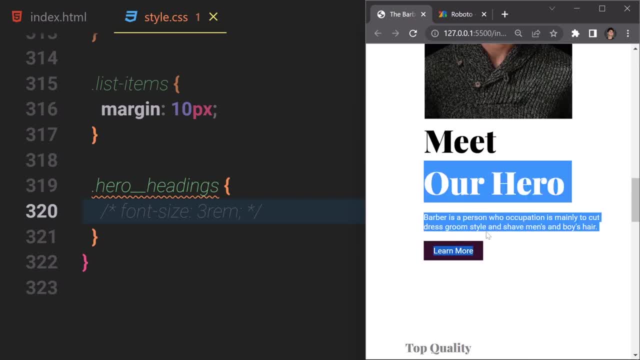 it will look like if you want to. it will look like, if you want to. i guess this is how it looks like and i, i guess this is how it looks like and i, i guess this is how it looks like and i guess, guess, guess, i'm gonna go with this style. i don't. 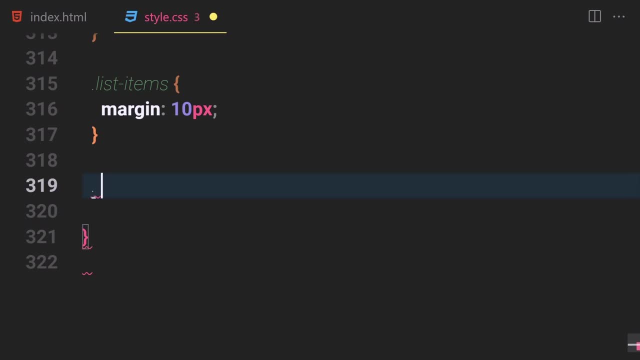 i'm gonna go with this style. i don't, i'm gonna go with this style. i don't have to increase or decrease the sizes, have to increase or decrease the sizes, have to increase or decrease the sizes of them, and let's just write or hero of them. and let's just write or hero. 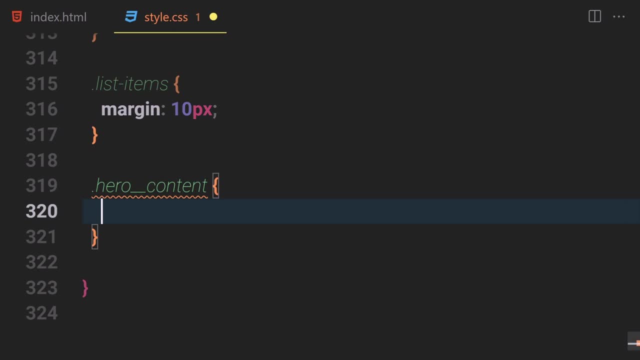 of them and let's just write: or hero dash dash content- c-o-n-t-e-n-t. dash dash content- c-o-n-t-e-n-t. dash dash content- c-o-n-t-e-n-t. and i'm going to provide a margin of zero, and i'm going to provide a margin of zero. 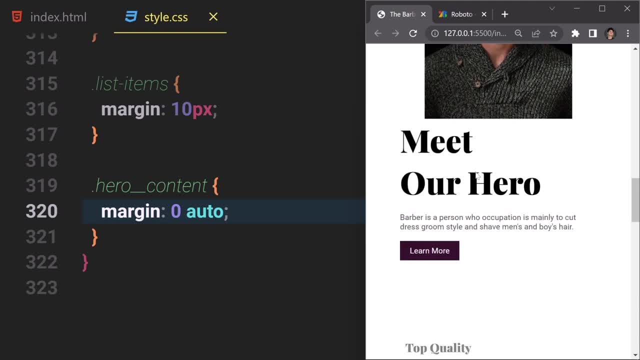 and i'm going to provide a margin of zero auto, so that everything is not only at auto, so that everything is not only at auto, so that everything is not only at the center, the center, the center. uh-huh, that's not working. uh-huh, that's not working. 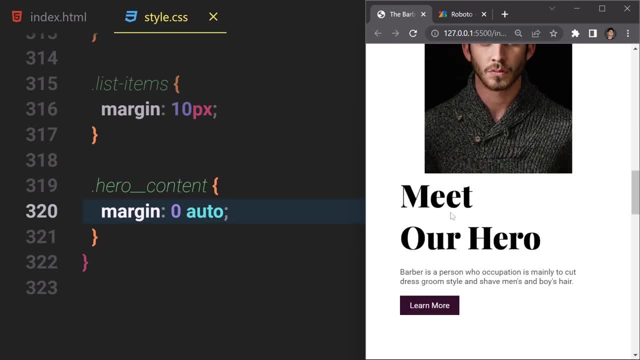 uh-huh, that's not working for the left and right. it's auto for the left and right. it's auto for the left and right. it's auto. uh-uh, you know what? uh-uh, you know what? uh-uh, you know what? this is going to be zero for the left and 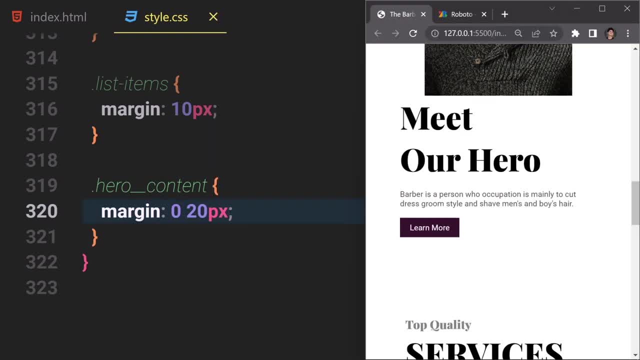 this is going to be zero for the left and this is going to be zero for the left and right. i'm going to give him like 20, right? i'm going to give him like 20, right? i'm going to give him like 20 pixel, maybe. 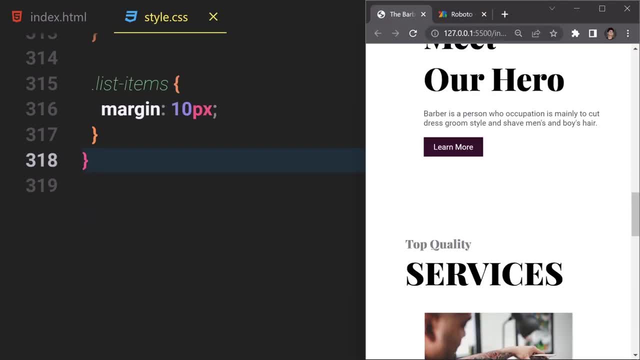 pixel maybe, pixel maybe. oh so, i'm going to remove that. oh so, i'm going to remove that. oh so, i'm going to remove that. that's looking okay in this case, we can. that's looking okay in this case, we can. that's looking okay in this case, we can also. we can also decrease the size of. 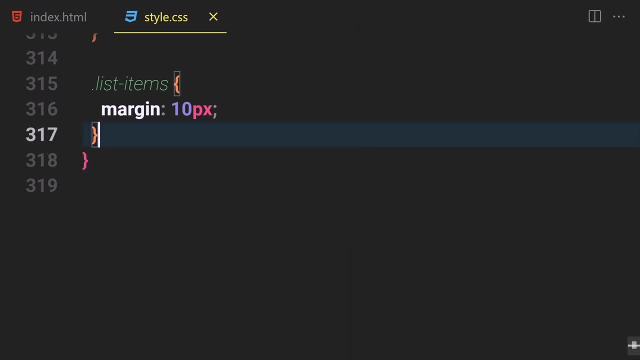 also, we can also decrease the size of. also. we can also decrease the size of this container. if you want to but for this container. if you want to but for this container if you want to, but for now it's looking totally okay. and now it's looking totally okay and. 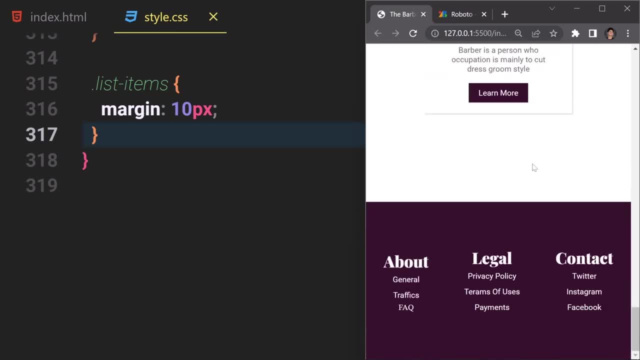 now it's looking totally okay. and services section- so what about it? this services section? so what about it? this services section? so what about it? this is also looking better, so i guess this is also looking better. so i guess this is also looking better. so i guess this is now like totally responsive, if you. 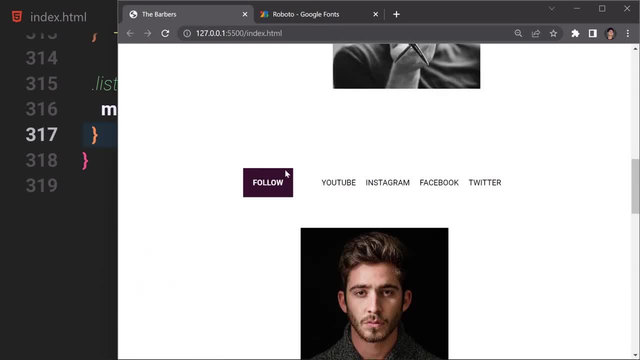 is now like totally responsive. if you is now like totally responsive, if you want to play around with this side, so want to play around with this side, so want to play around with this side, so totally do that if you want to. totally do that if you want to. 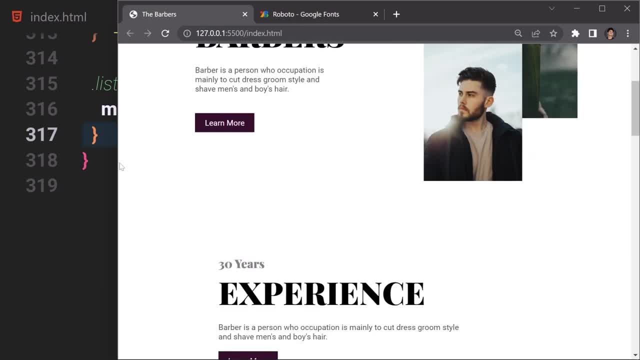 totally do that if you want to, okay. so in my case it's looking better, okay. so in my case, it's looking better, okay, so in my case, it's looking better in my machine, to be precise, in my machine, to be precise, in my machine, to be precise. uh, okay, so everything is working the way. 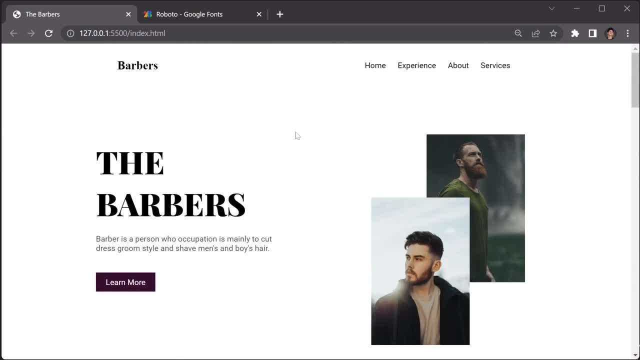 uh, okay, so everything is working the way. uh, okay, so everything is working the way we expand to work. so now we are totally, we expand to work. so now we are totally, we expand to work. so now we are totally done with this project and i will see. 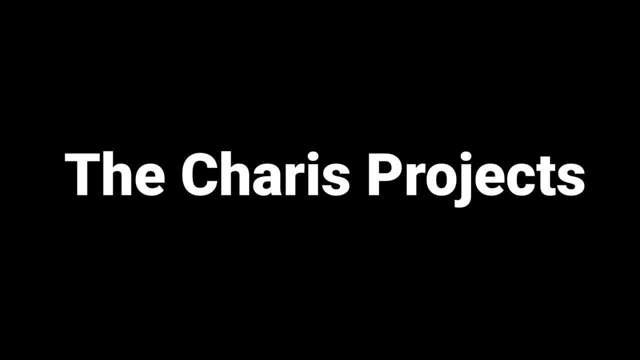 done with this project and i will see done with this project and i will see you in the next project. so bye, bye for you in the next project. so bye, bye for you in the next project. so bye, bye for now. all right, so before getting into the all right. so before getting into the all right, so before getting into the project, first of all, let me mention one project. first of all, let me mention one project. first of all, let me mention one thing. so if you want to use these same thing, so if you want to use these same, 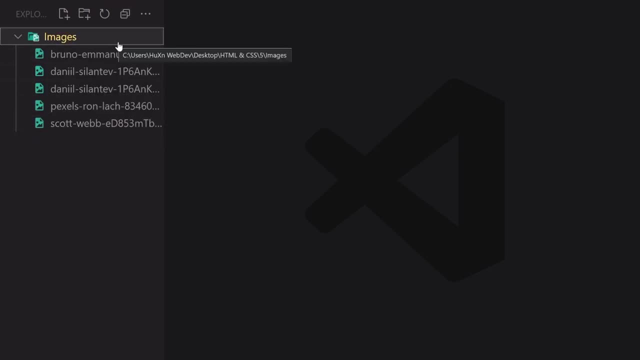 thing. so if you want to use these same images which i'm going to be using, images which i'm going to be using, images which i'm going to be using throughout this um project, so you can, throughout this um project, so you can throughout this um project, so you can. so i'm going to just create a new file. so i'm going to just create a new file. so i'm going to just create a new file. let me just zoom in a bit. i'm going to. let me just zoom in a bit. i'm going to. let me just zoom in a bit. i'm going to create a new file. give a name of like. 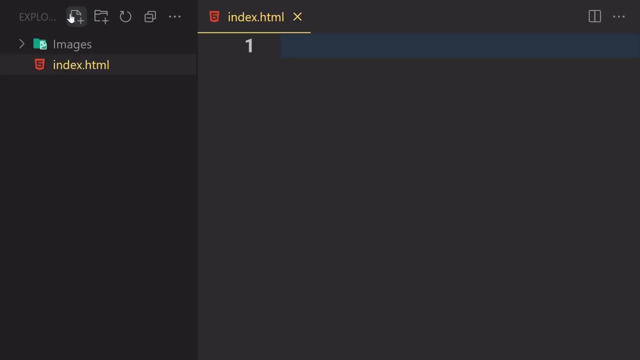 create a new file. give a name of like. create a new file. give a name of like: indexhtml. and now let's just create indexhtml. and now let's just create indexhtml. and now let's just create another one. give a name of like style. another one: give a name of like style. 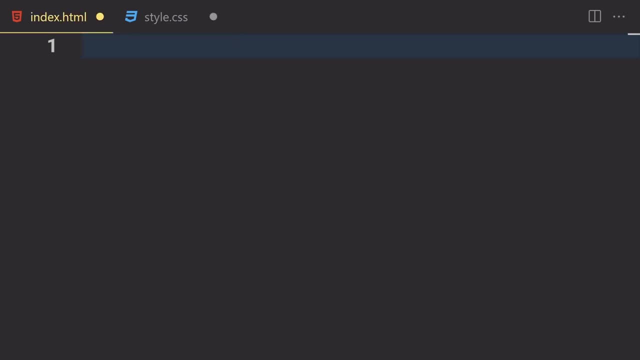 another one, give a name of like style: dot css for styling. all right, so in this dot css for styling, all right, so in this dot css for styling, all right, so in this indexhtml file, i'm going to just create indexhtml file, i'm going to just create. 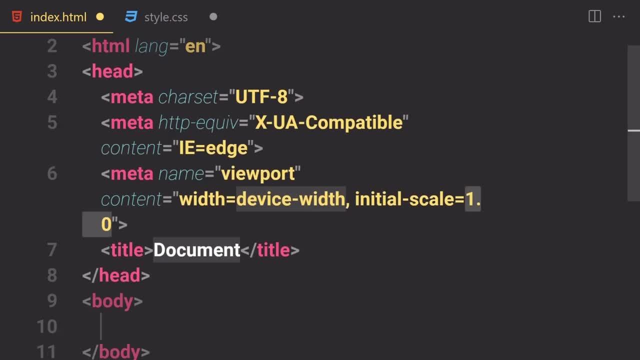 indexhtml file. i'm going to just create a doc type html first of all. so a doc type html first of all. so a doc type html first of all. so dot type html. so what do we have to do? i'm dot type html, so what do we have to do? i'm 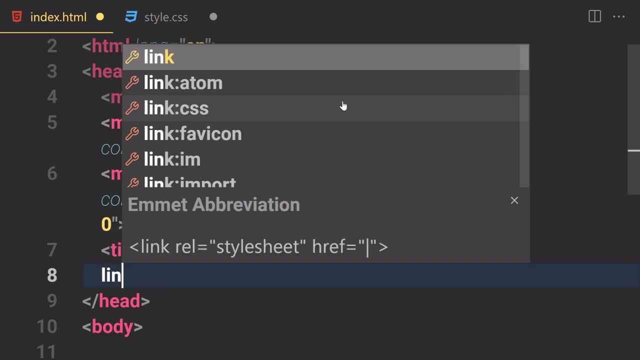 dot type html. so what do we have to do? i'm going to give a name of like, going to give a name of like, going to give a name of like- chairs, and i'm going to also uh link it- chairs, and i'm going to also uh link it. 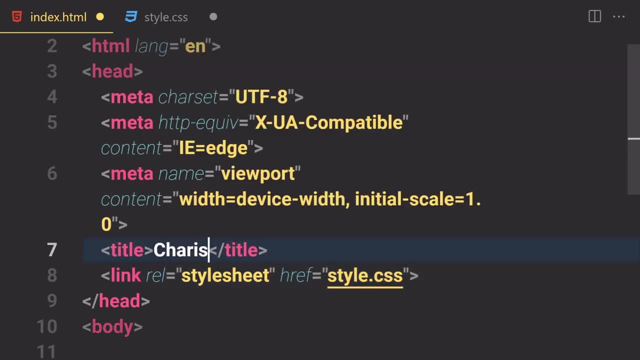 chairs, and i'm going to also, uh, link it with my css file as well. so i guess i with my css file as well. so i guess i with my css file as well. so i guess i messed it up something, messed it up something, messed it up something. so 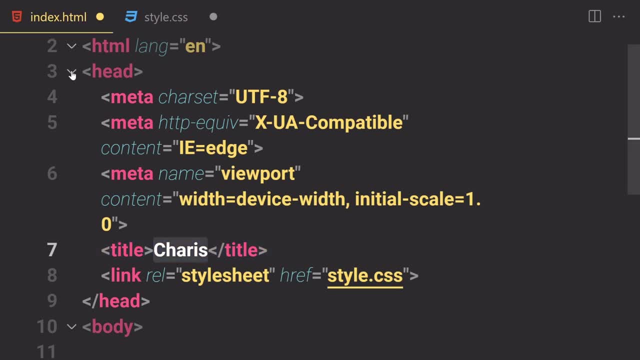 so so c-h-a-i-r-s. i guess that's fine. so now i'm c-h-a-i-r-s. i guess that's fine. so now i'm c-h-a-i-r-s. i guess that's fine. so now i'm going to just hide this heading area. 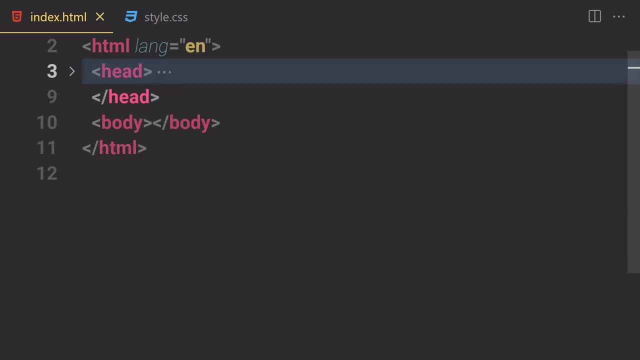 going to just hide this heading area. going to just hide this heading area or head area. now i'm going to right click or head area. now i'm going to right click or head area. now i'm going to right click on it and open it with a live server. so 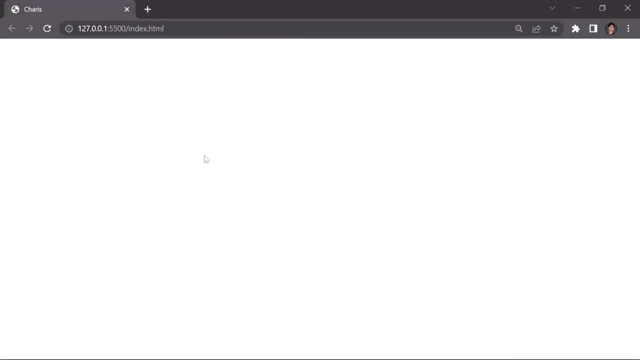 on it and open it with a live server. so, on it and open it with a live server. so it will now open it with a live server. it will now open it with a live server. it will now open it with a live server. so, all right, so we have nothing inside. 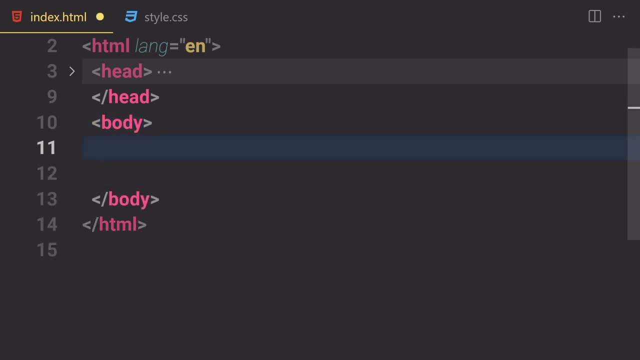 all right, so we have nothing inside. all right, so we have nothing inside our body and stuff. so now, let's just our body and stuff. so now, let's just our body and stuff. so now let's just get in towards first thing, so the first. get in towards first thing, so the first. 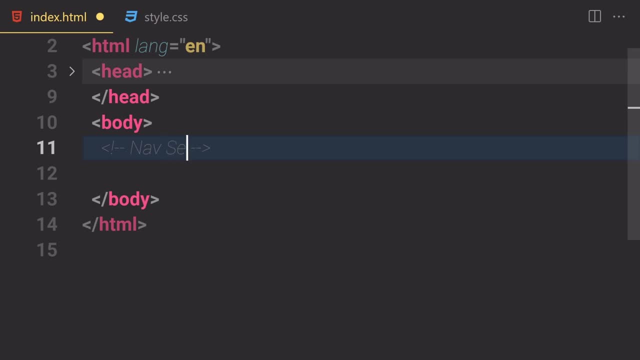 get in towards first thing. so the first thing which we are going to start, thing which we are going to start, thing which we are going to start, working on our nav, working on our nav, working on our nav, uh section start. so we are going to uh section start. so we are going to. 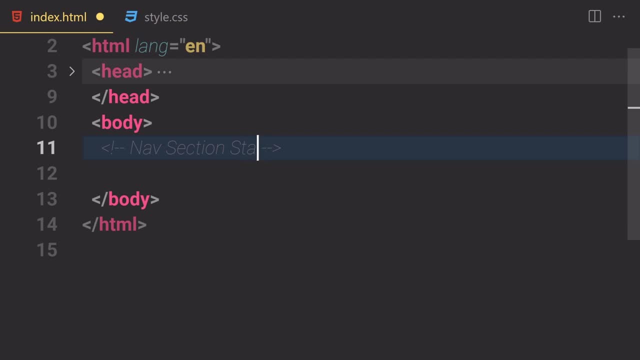 uh section start. so we are going to start working on our navigation area. start working on our navigation area. start working on our navigation area first of all. so i'm going to write like first of all. so i'm going to write like first of all. so i'm going to write like: nav str. oh, my goodness, str80. 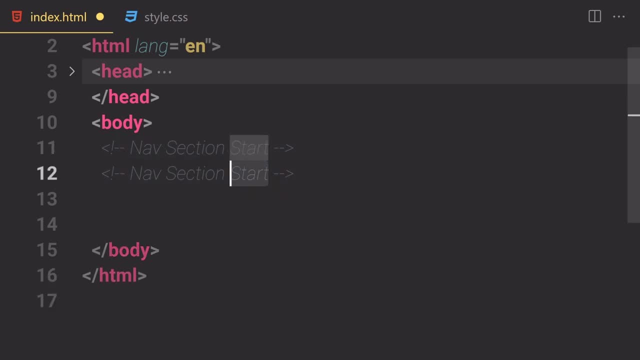 nav str. oh my goodness, str80 nav str. oh my goodness, str80 start art. so now let's just duplicate start art. so now let's just duplicate start art. so now let's just duplicate there and change this one to nav. there and change this one to nav. 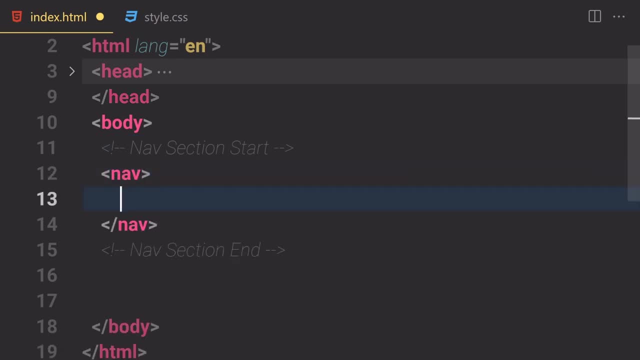 there and change this one to nav, section n and inside there we are going section n and inside there we are going section n and inside there we are going to be just writing our navigation inside, to be just writing our navigation inside, to be just writing our navigation inside. this navigation we are going to be. 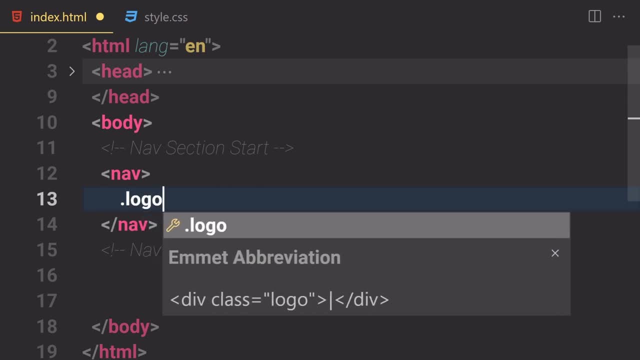 this navigation. we are going to be this navigation. we are going to be creating a div with the class of logo, creating a div with the class of logo, creating a div with the class of logo because we are going to be putting our, because we are going to be putting our. 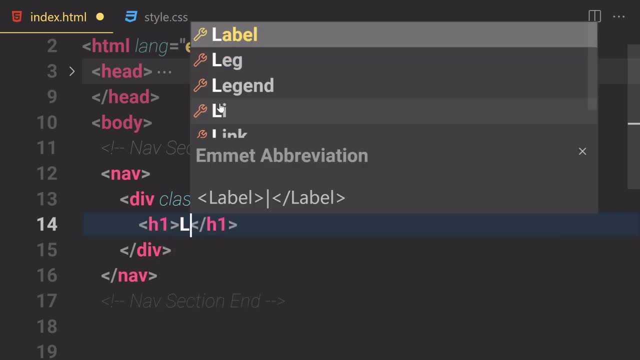 because we are going to be putting our logo inside this div now inside there. we logo inside this div, now inside there. we logo inside this div, now inside there. we are going to be just writing h1 with a. are going to be just writing h1 with a. 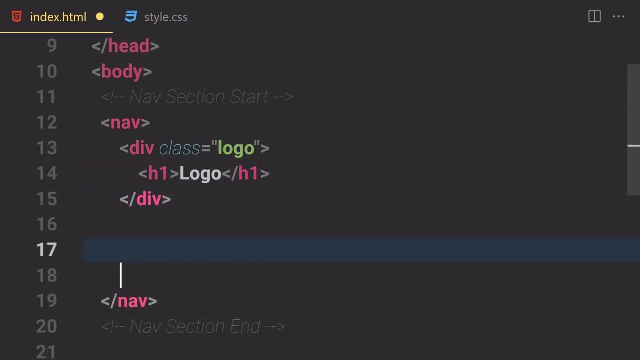 are going to be just writing h1 with a class, not a class, but as a label of logo. class, not a class, but as a label of logo. class, not a class, but as a label of logo. all right, so outside from there, i'm all right. so outside from there, i'm. 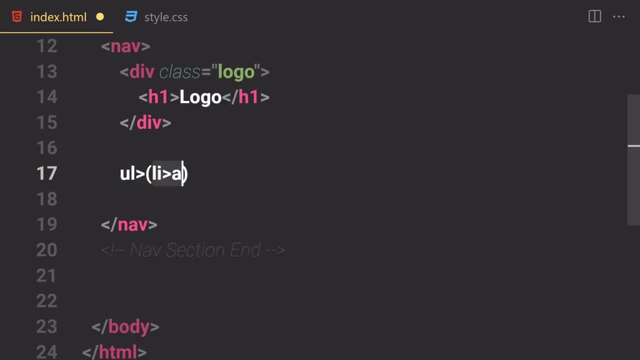 all right. so outside from there i'm gonna write a ul and then li, then anchor gonna write a ul and then li, then anchor gonna write a ul and then li, then anchor tag. and now let's just duplicate there tag. and now let's just duplicate there. tag. and now let's just duplicate there: uh, i guess four time would be fine. so, uh, i guess four time would be fine. so, uh, i guess four time would be fine. so i'm going to just duplicate that like. i'm going to just duplicate that like. 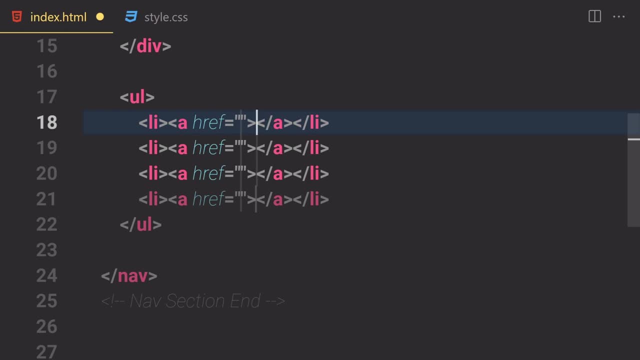 i'm going to just duplicate that like full time it will go to nowhere. so first, full time, it will go to nowhere. so first full time, it will go to nowhere. so first of all, we're going to be writing like of all. we're going to be writing like: 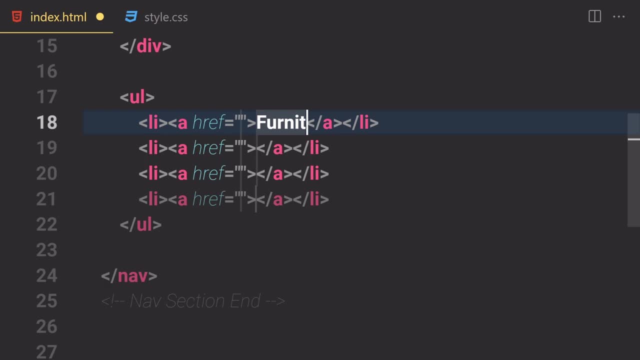 of all, we're going to be writing like furnitures. furniture will be fine and the second furniture will be fine, and the second furniture will be fine and the second will be project. the third one will be: i will be project. the third one will be i will be project. the third one will be, i guess, like a product will be fine and 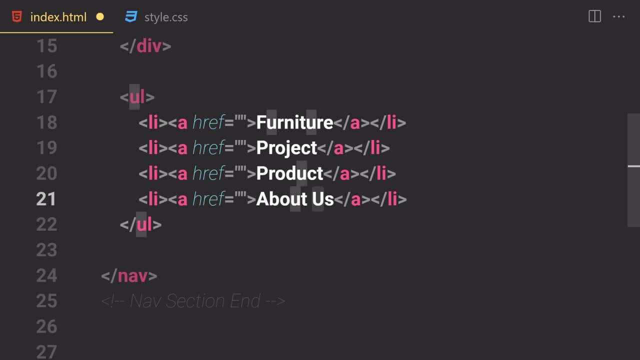 guess like a product will be fine. and guess like a product will be fine. and now let's just write over a bound a. now let's just write over a bound a. now let's just write over a bound, a section, or it should be like a, you know, 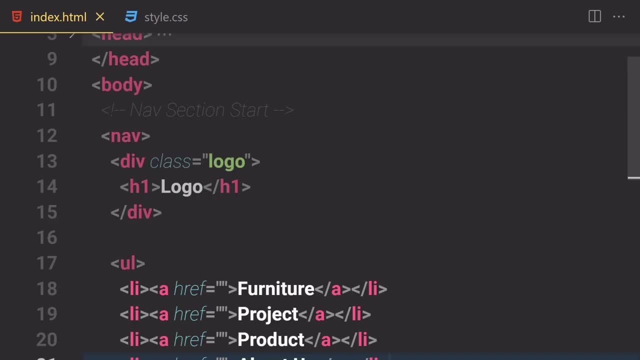 section, or it should be like a you know section, or it should be like a you know what uppercase would be fine. so if you, what uppercase would be fine. so if you, what uppercase would be fine. so if you save our file. so that's it now underneath. 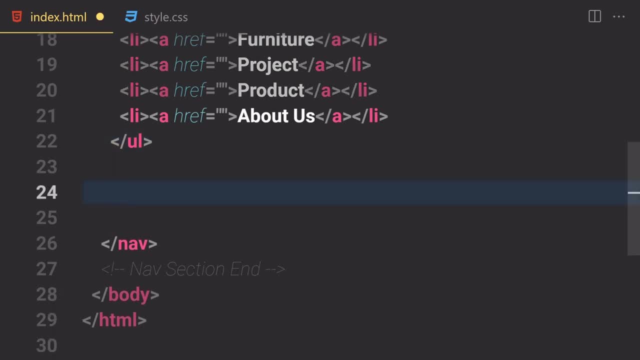 save our file. so that's it now underneath. save our file. so that's it now underneath this ul first of all. let's just try it. this ul first of all. let's just try it. this ul first of all. let's just try it: over button. so underneath this ul, let's. 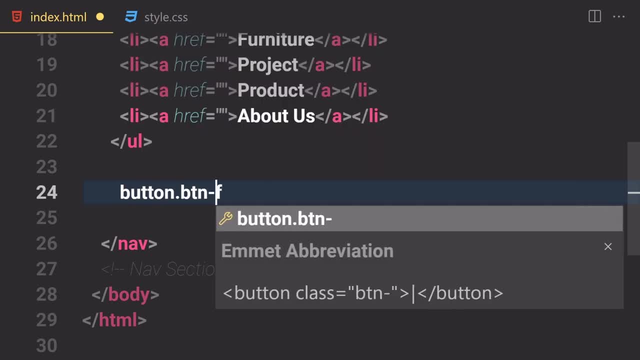 over button. so underneath this ul, let's over button. so underneath this ul, let's just create our button with the class of. just create our button with the class of. just create our button with the class of um btn and fill so learn not learn more um btn and fill so learn not learn more. 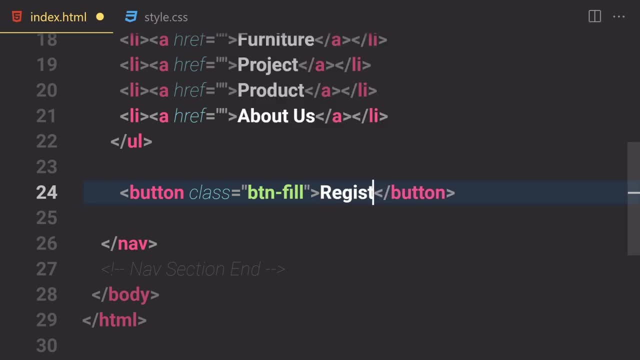 um, btn and fill. so learn, not learn more. but just register will be fine. but just register will be fine. but just register will be fine, uh, register, okay. so if you save our file, uh register okay. so if you save our file, uh register, okay. so if you save our file. so this is how currently things looks. 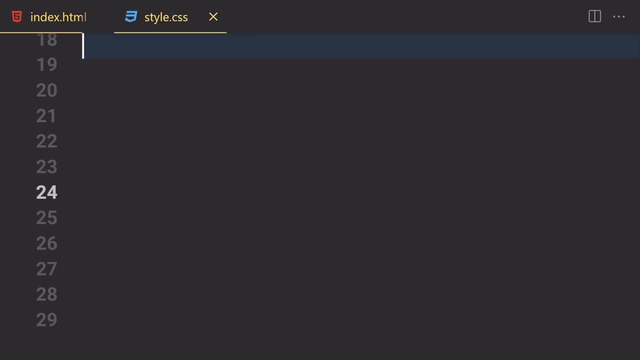 so this is how currently things looks. so this is how currently things looks like. so now let's jump into our css and like: so now let's jump into our css and like: so now let's jump into our css, and now let's just style that a bit. so what? now, let's just style that a bit. so what? now let's just style that a bit. so what do we have to do? i'm going to remove. do we have to do? i'm going to remove. do we have to do? i'm going to remove everything from here. and now, let's just 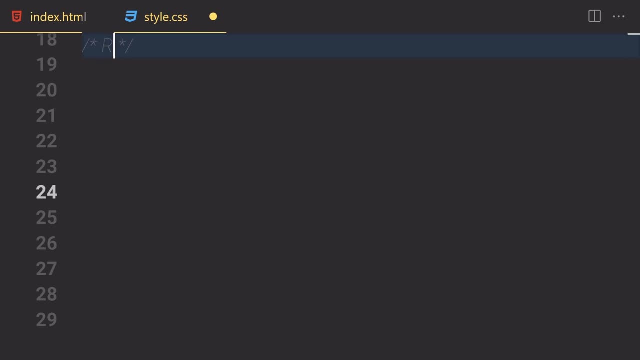 everything from here and now. let's just everything from here and now. let's just start working on a reset. so i'm going start working on a reset. so i'm going start working on a reset. so i'm going to write a comment for myself, like a. 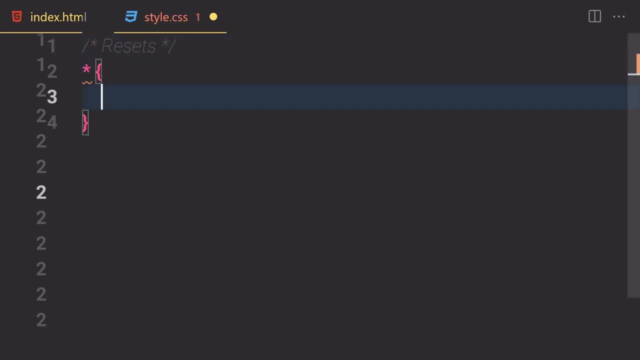 to write a comment for myself like a. to write a comment for myself like a: resets, and let's just start working on resets. and let's just start working on resets and let's just start working on our everything selector margin will be. our everything selector margin will be. 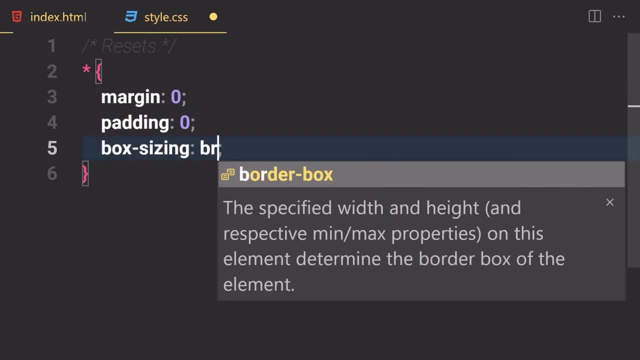 our everything selector margin will be zero, padding will be also zero and box zero padding will be also zero and box zero padding will be also zero and box sizing will be now set to border box. sizing will be now set to border box. sizing will be now set to border box. so this is going to be it for the reset. 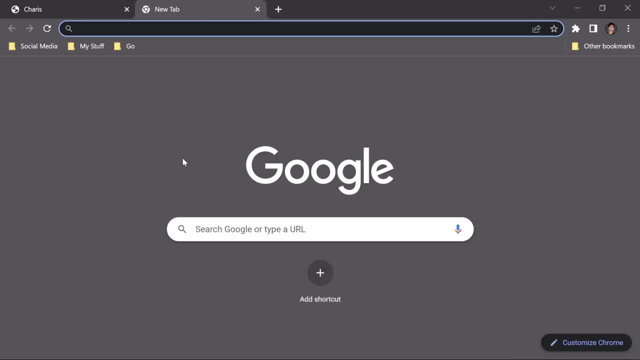 so this is going to be it for the reset. so this is going to be it for the reset. so what else do we have to do? we have to. so what else do we have to do? we have to. so what else do we have to do? we have to get a fonts from, or um, fontsgooglecom. 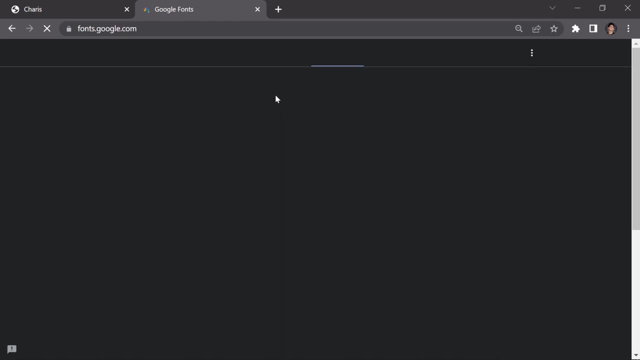 get a fonts from or um fontsgooglecom. get a fonts from or um fontsgooglecom. so we have to just go to this fonts. so we have to just go to this fonts. so we have to just go to this fonts googlecom. and here we are going to be. 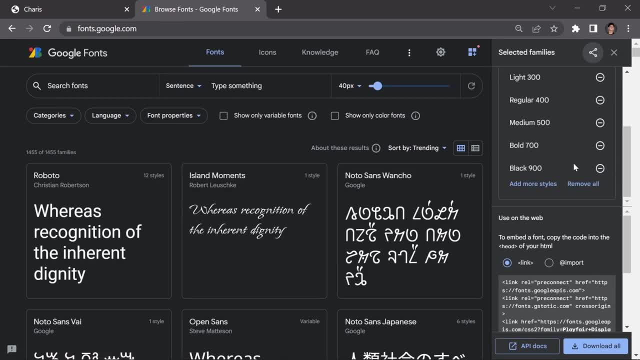 googlecom. and here we are going to be googlecom, and here we are going to be just getting one font car a play fire, or just getting one font car a play fire, or just getting one font car a play fire or play fair, whatever you want to call that. 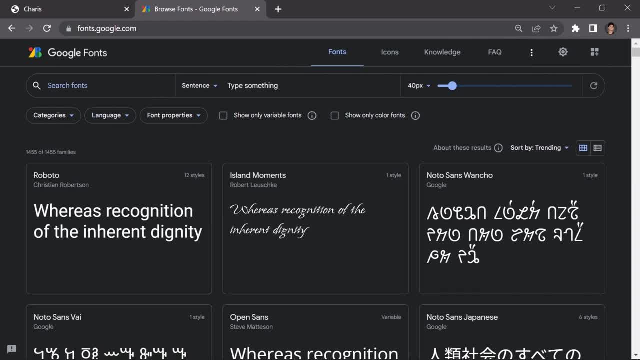 play fair, whatever you want to call that. play fair, whatever you want to call that. i'm going to remove these other fonts. i'm going to remove these other fonts. i'm going to remove these other fonts which we use in our previous projects, so which we use in our previous projects, so. 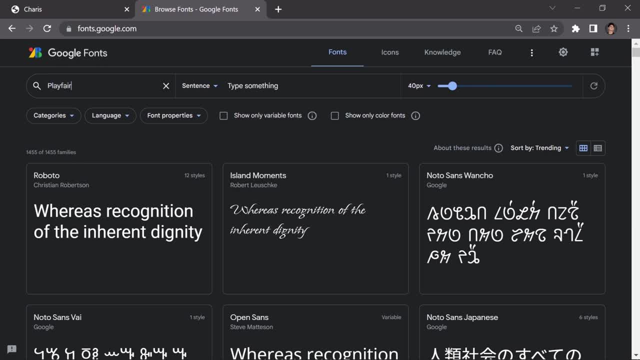 which we use in our previous projects. so now, in this case, what i'm going to do now in this case, what i'm going to do now in this case, what i'm going to do, i'm going to just search for a play fire. i'm going to just search for a play fire. 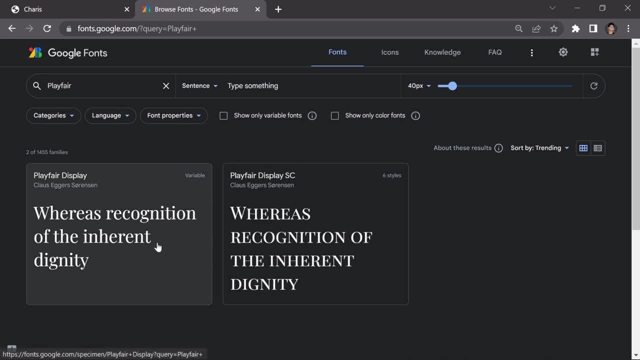 i'm going to just search for a play fire or play fair display, whatever you want, or play fair display, whatever you want, or play fair display, whatever you want to call that. so i'm going to just click to call that. so i'm going to just click. 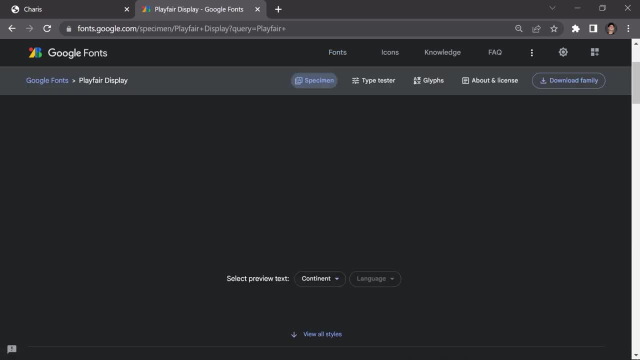 to call that. so i'm going to just click on this um this first one. and now let's on this, um this first one. and now let's on this um this first one, and now let's just select. i guess i'm going to select, just select. i guess i'm going to select. 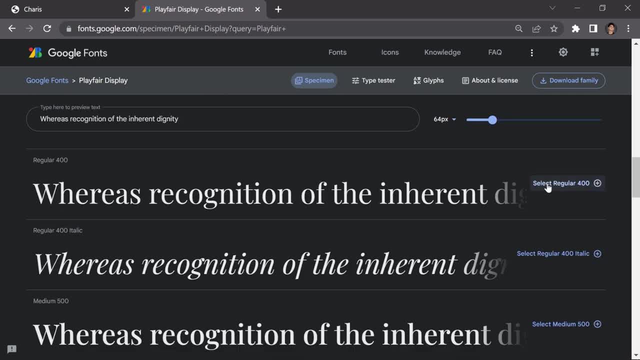 just select. i guess i'm going to select everything, everything, everything. all of its styling, but not italic one. all of its styling, but not italic one. all of its styling, but not italic one, but a regular one would be fine, but a regular one would be fine, but a regular one would be fine. so 500. then we have 600, 700. 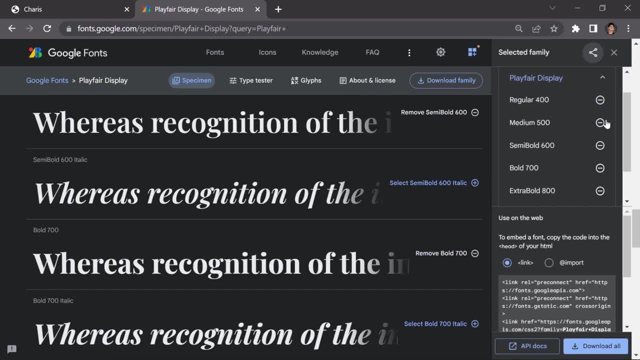 so 500. then we have 600, 700, 800, so 500, then we have 600, 700, 800 and 900, so now you have to just click and 900. so now you have to just click and 900. so now you have to just click on that. and now let's just click on this. 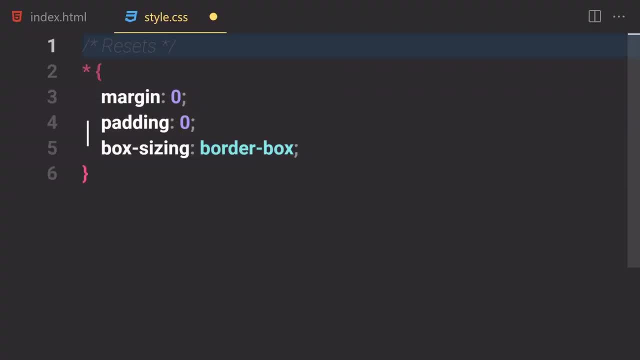 on that, and now let's just click on this, on that. and now let's just click on this: import, import, import. and let's just copy this link, and i'm, and let's just copy this link, and i'm, and let's just copy this link and i'm gonna put it above, and now let's just 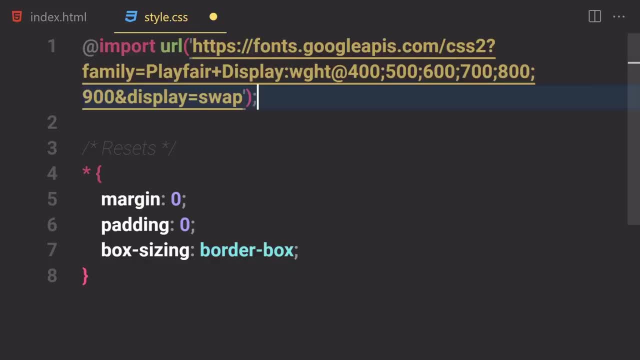 gonna put it above, and now, let's just gonna put it above, and now let's just copy, copy, copy: display, fire display, or whatever you display fire display, or whatever you display fire display, or whatever you want to call that, want to call that, want to call that, and i'm going to put it inside my root. and i'm going to put it inside my root. and i'm going to put it inside my root. or you know, i'm going to paste it right. or you know, i'm going to paste it right. or you know, i'm going to paste it right here and i'm going to comment there. for 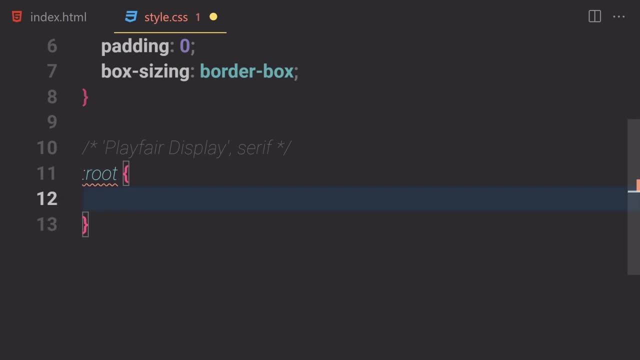 here and i'm going to comment there for here, and i'm going to comment there for a second, a second, a second, and now let's just start working on, or, and now let's just start working on, or, and now let's just start working on, or variables. so the first variable which i'm 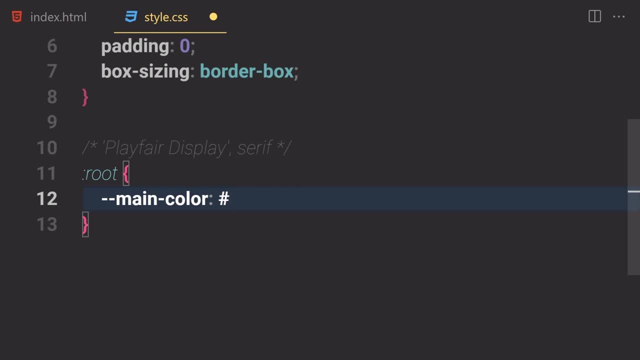 variables. so the first variable which i'm variables, so the first variable which i'm going to be creating is a main color. going to be creating is a main color going to be creating is a main color. so we are going to be using this color. so we are going to be using this color. 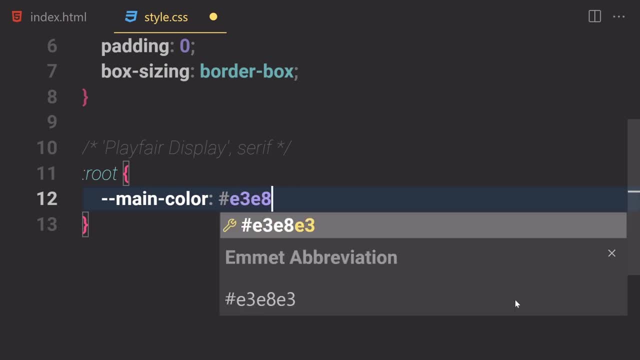 so we are going to be using this color throughout, so which is e3e, throughout, so which is e3e throughout, so which is e3e: uh eight e four. i guess that was the uh eight e four. i guess that was the uh eight e four. i guess that was the color. color, color and kind of a grayish color, so now let's. and kind of a grayish color, so now let's. and kind of a grayish color. so now let's just create a new color which is a. just create a new color which is a. 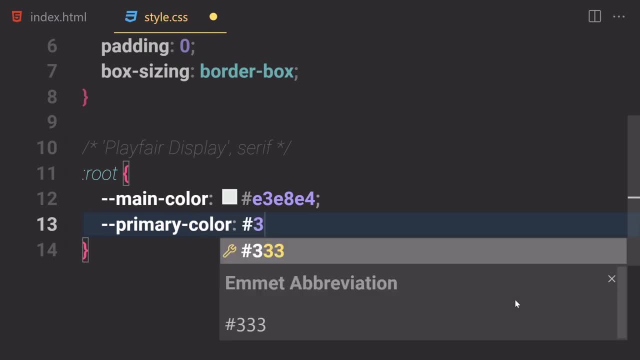 just create a new color which is a primary color, so this is going to be now primary color. so this is going to be now primary color. so this is going to be now like three, six, three, six and three, six. like three, six, three, six and three, six. 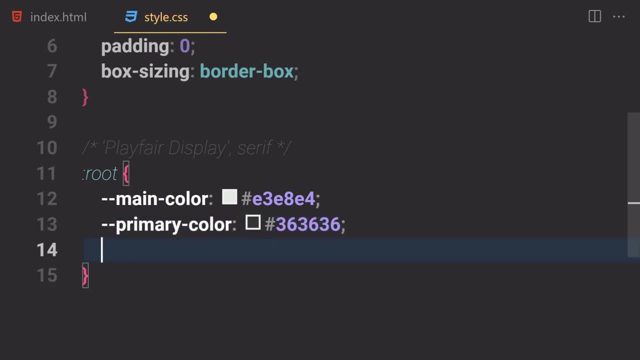 like three, six, three, six and three, six. yeah, that's going to be fine. yeah, that's going to be fine. yeah, that's going to be fine. a little bit darker gray, then we have a a little bit darker gray, then we have a a little bit darker gray, then we have a main form, so main font, which will be: main form, so main font, which will be main form, so main font, which will be that font. so i'm going to comment that that font. so i'm going to comment that that font. so i'm going to comment that i'm going to cut it from there. i'm going 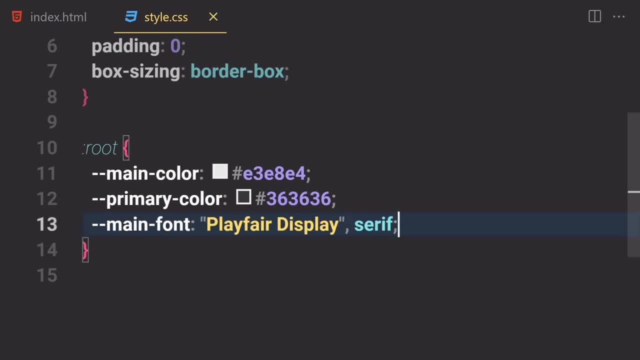 i'm going to cut it from there. i'm going, i'm going to cut it from there, i'm going to paste it right here. so if you to paste it right here, so if you to paste it right here, so if you save a file, so these are it for all. 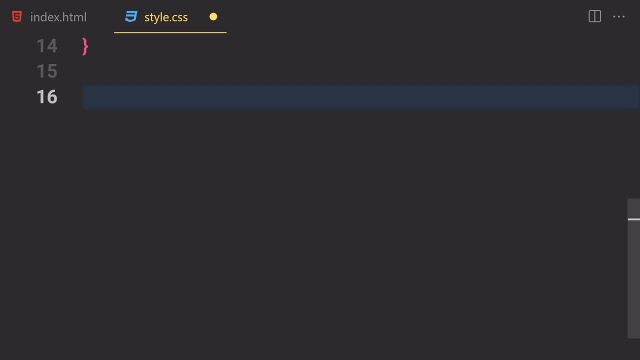 save a file, so these are it for all. save a file, so these are it for all. variables- okay, or custom properties- variables- okay, or custom properties- variables- okay, or custom properties- whatever you want to call that, now let's. whatever you want to call that, now let's. 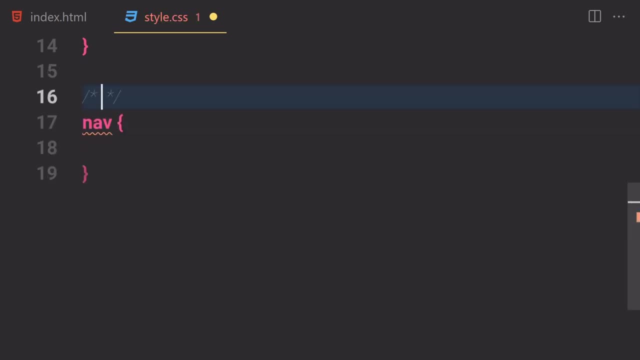 whatever you want to call that. now let's just start working on our navigation. but just start working on our navigation. but just start working on our navigation. but before we do, i'm going to have to write. before we do, i'm going to have to write. before we do, i'm going to have to write a comment for myself, like a nav. 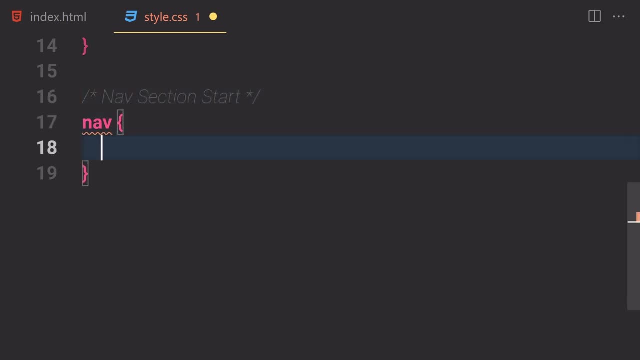 a comment for myself like a nav. a comment for myself like a nav: section start: okay, so this is going to be section. okay, so this is going to be section. okay, so this is going to be the comment. and now inside there, what do we? the comment. and now inside there, what do we? the comment. and now inside there, what do we have to do? we are going to be first of have to do. we are going to be first of have to do. we are going to be, first of all, writing a display of flags justify all. writing a display of flags justify. 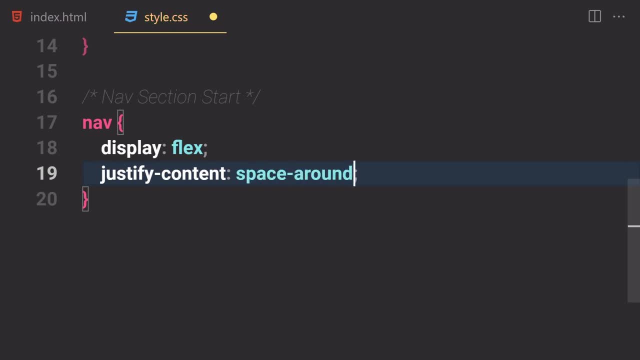 all writing a display of flags. justify content will be now set to not center. content will be now set to not center. content will be now set to not center, but just a space around. and now let's, but just a space around. and now let's, but just a space around. and now let's just write a line items and it will be. 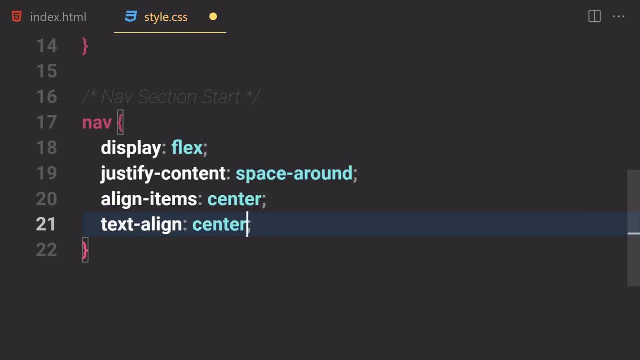 just write a line items and it will be. just write a line items and it will be now set to center and text align will be now set to center and text align will be now set to center and text align will be also set to center. okay, so font family. also set to center. okay, so font family also set to center. okay, so font family. i'm going to change that to like not. i'm going to change that to like not. i'm going to change that to like not water. but i guess i'm going to just 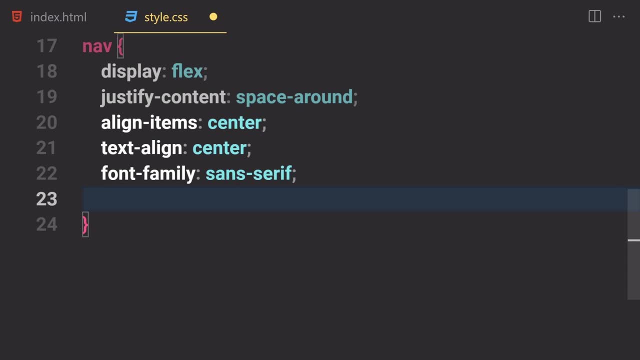 water, but i guess i'm going to just water, but i guess i'm going to just change that to sensor would be fine. you change that to sensor would be fine. you change that to sensor would be fine. you can choose whichever kind of form. you can choose whichever kind of form you. 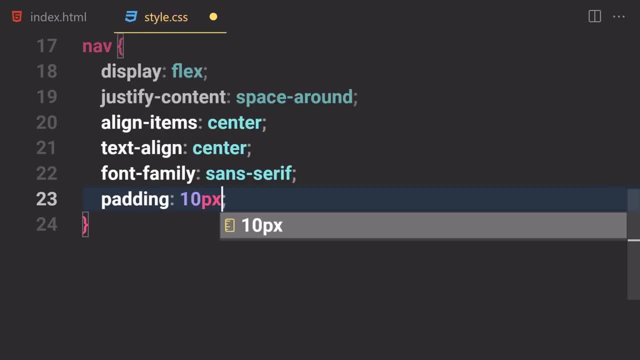 can choose whichever kind of form you like, but in my case, sensor would be fine, like, but in my case, sensor would be fine, like, but in my case sensor would be fine. so, padding, i'm going to give like 10. so, padding, i'm going to give like 10. 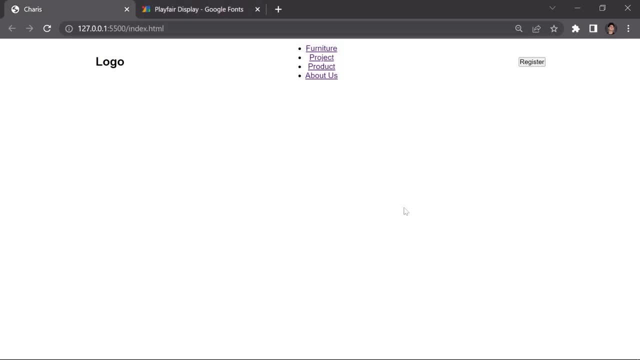 so, padding, i'm going to give like 10 pixel all around, and now if you save pixel all around, and now if you save pixel all around, and now if you save that, and now let's just preview it so that, and now let's just preview it so. 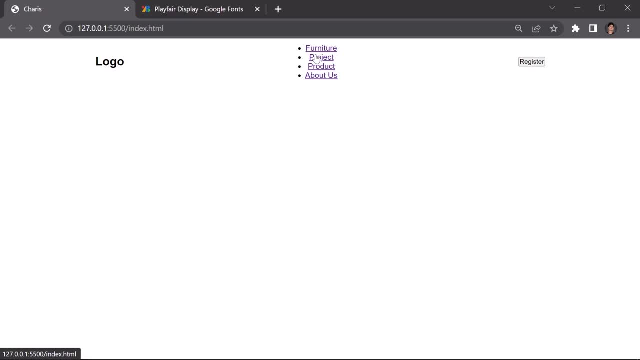 that, and now let's just preview it. so it's looking cool. it's looking cool. it's looking cool, but we have to take care of these. so we, but we have to take care of these, so we, but we have to take care of these. so we want to set that to the inline style. so 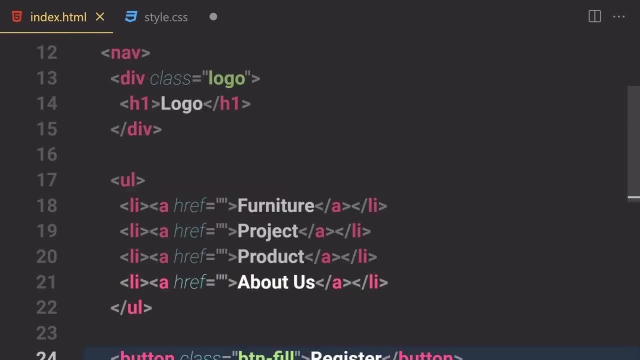 want to set that to the inline style. so want to set that to the inline style. so what do we have to do for that? first of what do we have to do for that? first of what do we have to do for that? first of all, we want to select this ul. i mean 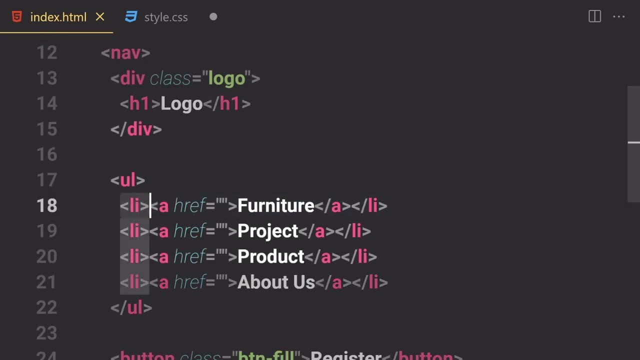 all we want to select this ul. i mean all we want to select this ul. i mean, like this li which is inside this ul, so like this li which is inside this ul, so like this li which is inside this ul, so we want to select that. so for that first, 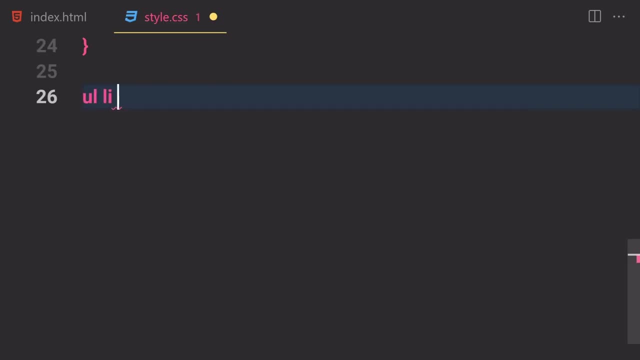 we want to select that. so for that first. we want to select that. so for that, first of all. we are going to be writing a ul of all. we are going to be writing a ul of all. we are going to be writing a ul. then, inside this ul, we have our allies. 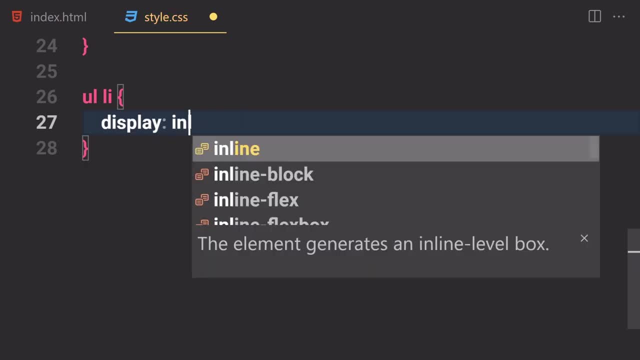 then inside this ul, we have our allies, then inside this ul, we have our allies. so now we select there. now, let's just so. now we select there. now, let's just so. now we select there. now let's just write a display of inline. okay, so, write a display of inline, okay so. write a display of inline. okay, so if you just say that you know i'm going, if you just say that you know i'm going, if you just say that you know i'm going to just save this file, and now it's to just save this file, and now it's. 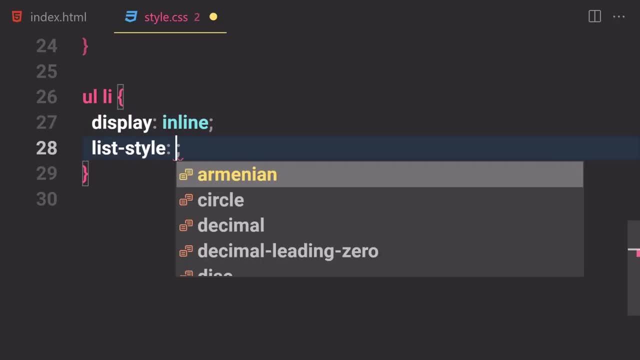 to just save this file. and now it's looking cool, but now also remove that looking cool. but now also remove that looking cool, but now also remove that list style. and now let's just set that list style. and now let's just set that list style, and now let's just set that to none. and if you say that that wasn't, 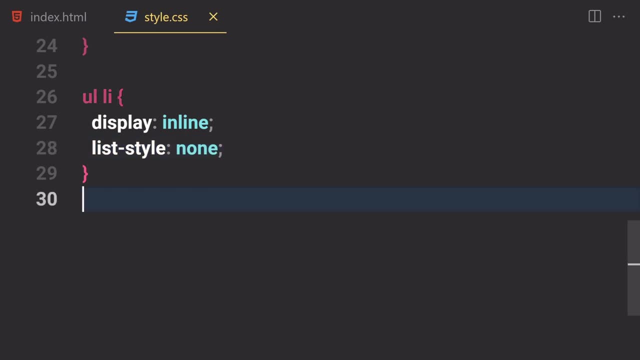 to none. and if you say that that wasn't to none, and if you say that that wasn't showing up, showing up, showing up, but we still remove that anyways. so now, but we still remove that anyways. so now, but we still remove that anyways. so now, let's just start working on over each of. 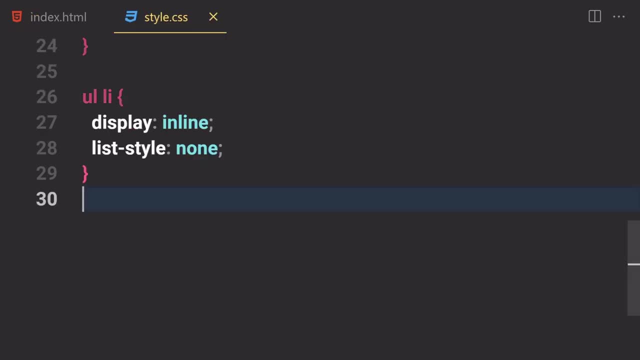 let's just start working on over each of. let's just start working on over each of these anchor tags, which is right here, so these anchor tags, which is right here, so these anchor tags, which is right here, so now let's just select that. so, if you, 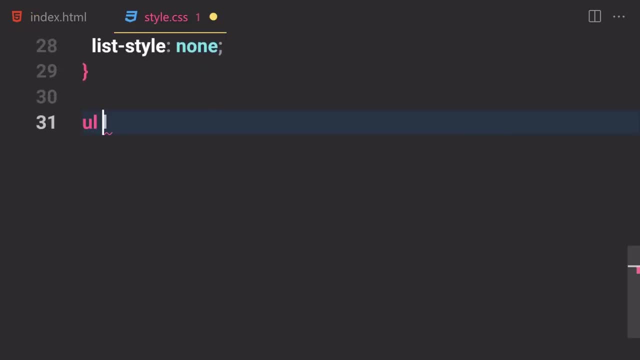 now, let's just select that. so if you now, let's just select that. so if you want to select that, want to select that, want to select that, first of all, we are going to be using a. first of all, we are going to be using a. first of all, we are going to be using a ul, then li and then anchor tags. so now, 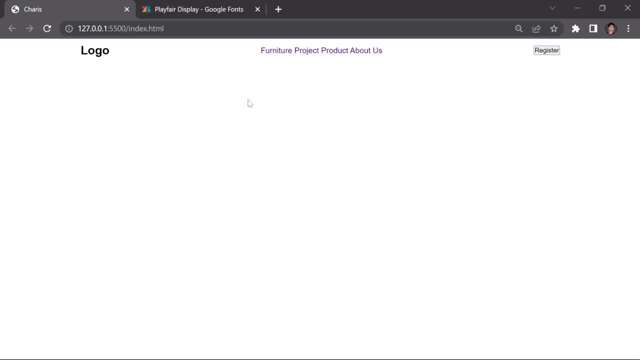 ul, then li and then anchor tags. so now ul, then li and then anchor tags. so now i'm going to just write a text, i'm going to just write a text. i'm going to just write a text, declaration and none. so it will not. declaration and none, so it will not. 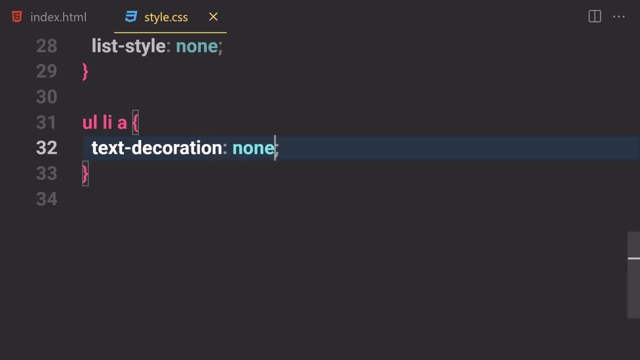 declaration and none, so it will not remove their text decoration from these. remove their text decoration from these. remove their text decoration from these- uh anchor tags and what else do we have? uh anchor tags and what else do we have? uh anchor tags and what else do we have to do? we are going to be also changing. 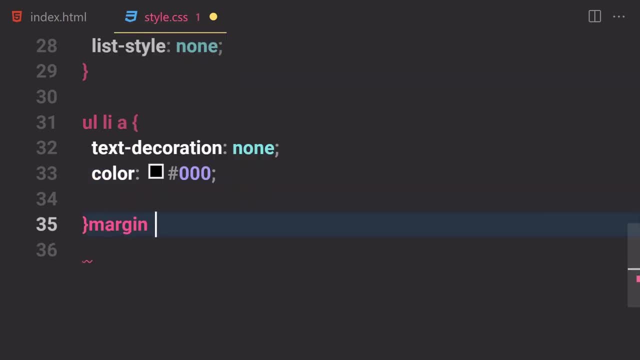 to do. we are going to be also changing to do. we are going to be also changing the color to be totally black and margin the color to be totally black and margin the color to be totally black and margin for the left area. oh, my goodness, what am? 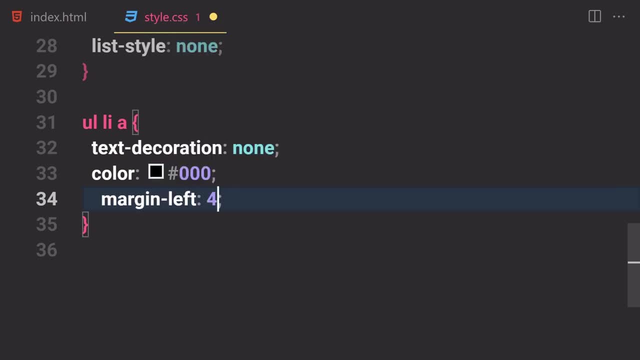 for the left area? oh my goodness, what am for the left area? oh my goodness, what am i even doing some merging for the lift? i'm even doing some merging for the lift. i'm even doing some merging for the lift. uh, i'm gonna give him like four remote 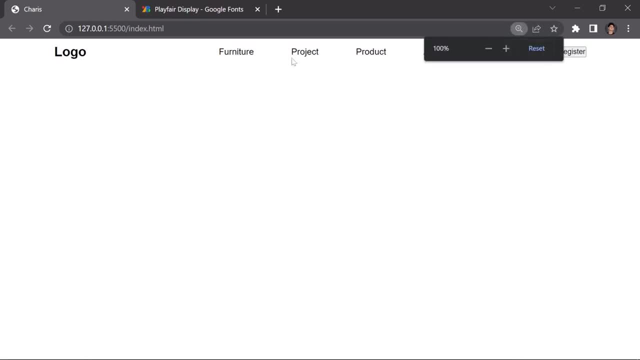 uh, i'm gonna give him like four remote. uh, i'm gonna give him like four remote to be fine. and now if you sell that, to be fine. and now if you sell that, to be fine. and now if you sell that and these are looking cool, you know so. and these are looking cool. you know so. and these are looking cool, you know so. these are looking cool now. what else do these are looking cool now. what else do these are looking cool now? what else do we have to do? i'm going to also provide. we have to do. i'm going to also provide. 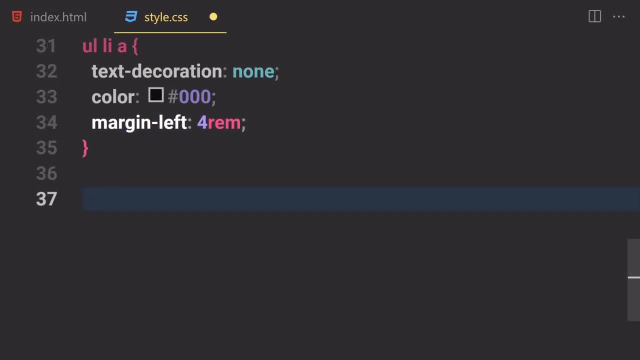 we have to do. i'm going to also provide a hover effect on that as well. so for a hover effect on that as well. so for a hover effect on that as well. so for there, let me just select that uli, and there, let me just select that uli, and 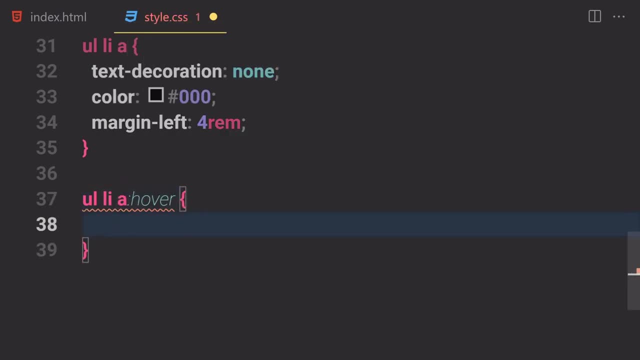 there, let me just select that uli and anchor tag one more time. and now let's anchor tag one more time. and now let's anchor tag one more time. and now let's just use that hover effect on that. so just use that hover effect on that. so. 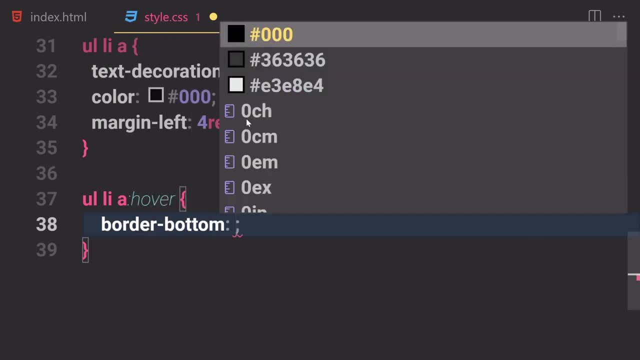 just use that hover effect on that. so once we hold our mouse over to it, so we, once we hold our mouse over to it, so we, once we hold our mouse over to it, so we want to provide a border for the bottom, want to provide a border for the bottom. 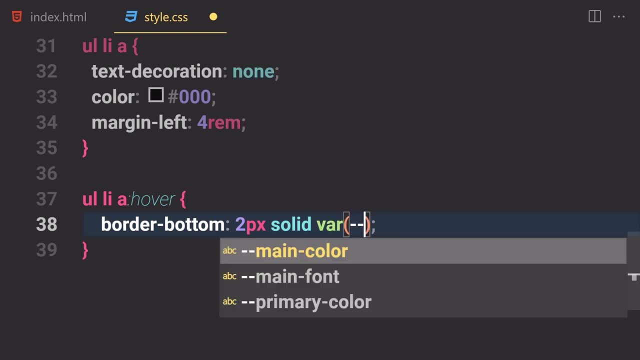 want to provide a border for the bottom, to like two pixel and solid. and now to like two pixel and solid, and now to like two pixel and solid, and now let's just use. or what let's just use, let's just use, or what let's just use. 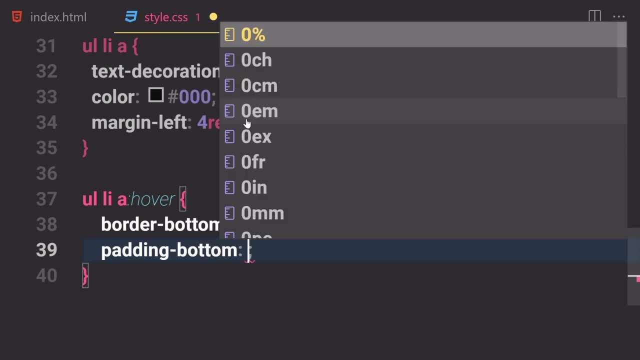 let's just use- or what? let's just use- our primary color. so padding for the, our primary color. so padding for the, our primary color. so padding for the bottom. i'm going to give him like 10 bottom. i'm going to give him like 10. 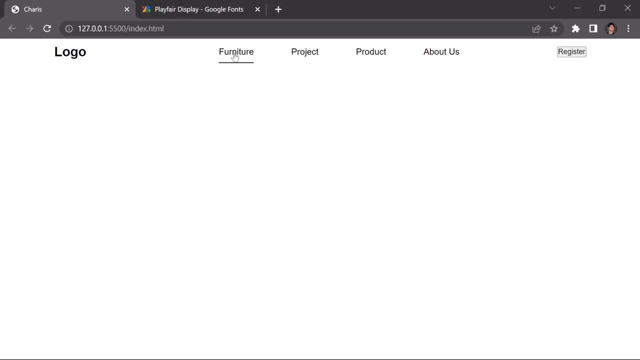 bottom. i'm going to give him like 10 pixel and knife is there. pixel and knife is there. pixel and knife is there. and now if you hold our mouse over to, and now if you hold our mouse over to, and now if you hold our mouse over to it. so here you can see. we are now getting it. so here you can see, we are now getting it. so here you can see, we are now getting that border bottom right here, okay, so that border bottom right here, okay, so that border bottom right here, okay. so now let's just take care of this. now let's just take care of this. 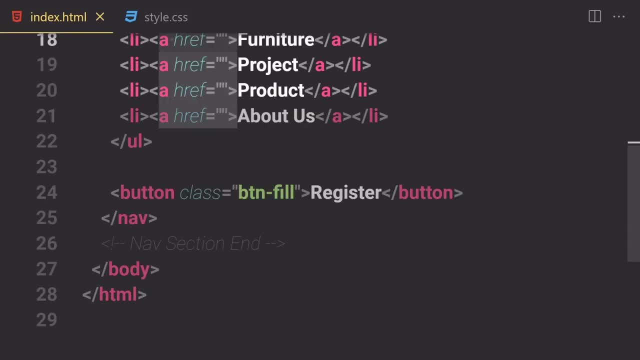 now let's just take care of this. register bound real quick. so what was register bound real quick? so what was register bound real quick? so what was the class? the class was btn fill, so i'm the class. the class was btn fill, so i'm the class. the class was btn fill, so i'm gonna copy that from here and i'm gonna. 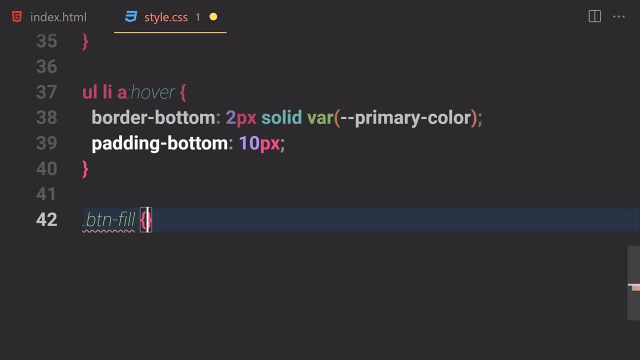 gonna copy that from here, and i'm gonna gonna copy that from here and i'm gonna just paste it right here. so let's just just paste it right here. so let's just just paste it right here. so let's just select that btn fill. select that btn fill. 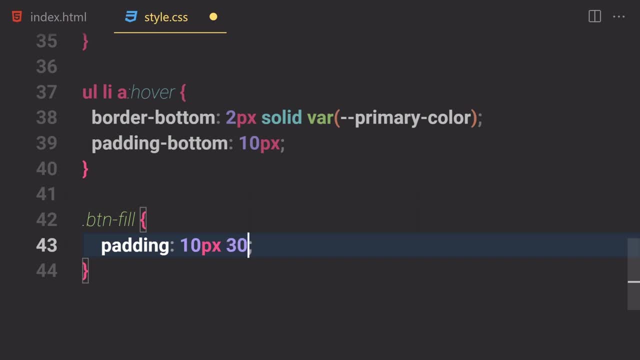 select that btn fill and i'm going to just provide a padding of and i'm going to just provide a padding of, and i'm going to just provide a padding of like 10 pixel for top and bottom, like 10 pixel for top and bottom, like 10 pixel for top and bottom, 30 pixel for the left and right, and i'm 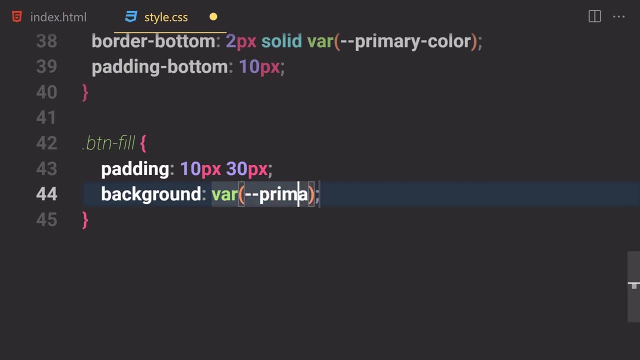 30 pixel for the left and right and i'm 30 pixel for the left and right and i'm going to also change the background. going to also change the background, going to also change the background color to be like a war of their primary color, to be like a war of their primary. 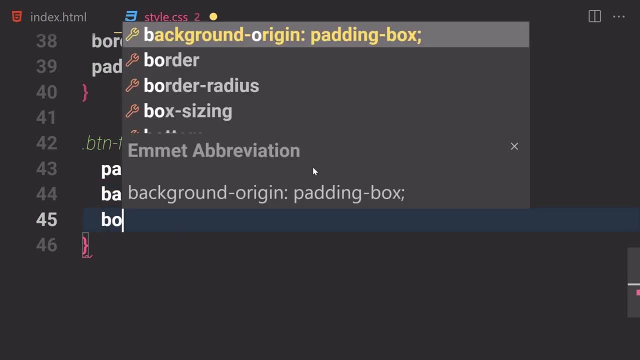 color to be like a war of their primary color, which we declare, and also let's color which we declare. and also let's color which we declare. and also let's just use a border to be like none. just use a border to be like none. just use a border to be like none, because we want to remove their ugly. 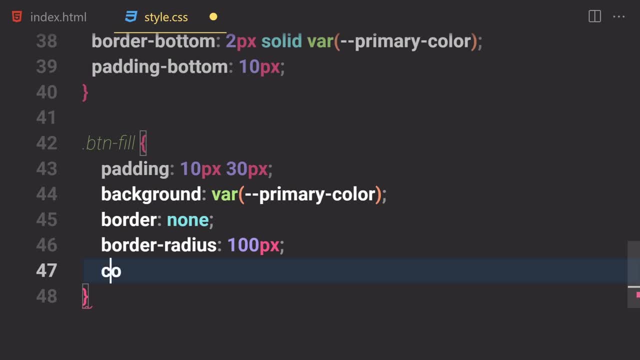 because we want to remove their ugly, because we want to remove their ugly border. and now let's just set the border border. and now let's just set the border border. and now let's just set the border radius to be 100 pixel and color not. radius to be 100 pixel and color not. 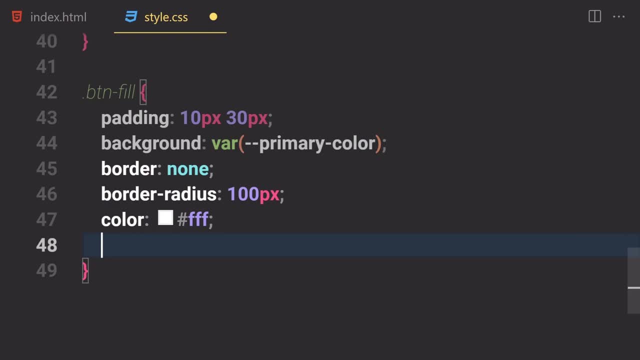 radius to be 100 pixel and color: not columns but color. in this case, we are columns but color. in this case, we are columns but color. in this case, we are going to be setting that to like totally, going to be setting that to like, totally, going to be setting that to like totally pure white and cursor will be pointer. so 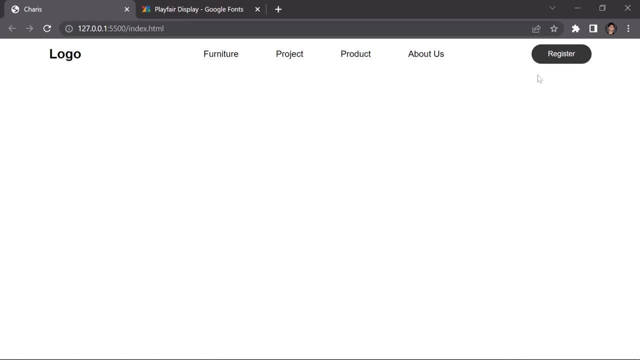 pure white and cursor will be pointer. so pure white and cursor will be pointer. so if you save that and here you can see, if you save that and here you can see, if you save that and here you can see, this is how our button looks like. so if 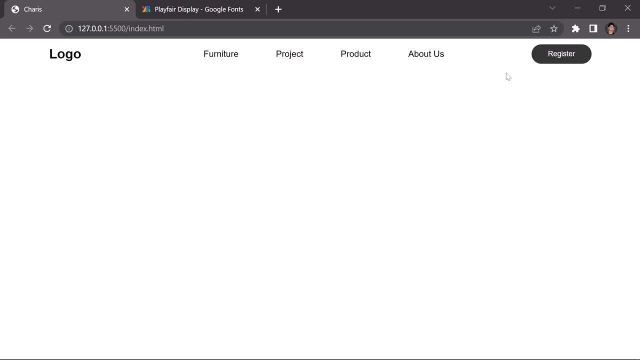 this is how our button looks like. so, if this is how our button looks like. so if you have a mouse ordered, so we are just. you have a mouse ordered, so we are just. you have a mouse ordered, so we are just getting that cursor button. cursor of. 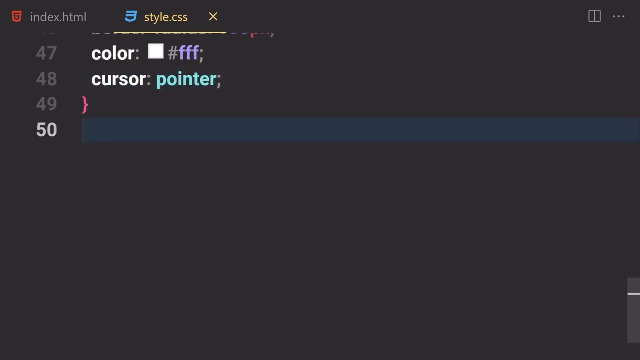 getting that cursor button, cursor of getting that cursor button, cursor of pointer to be precise, pointer to be precise, pointer to be precise. so now we are totally done with this. so now we are totally done with this. so now we are totally done with this navigation as well. so now, section end. 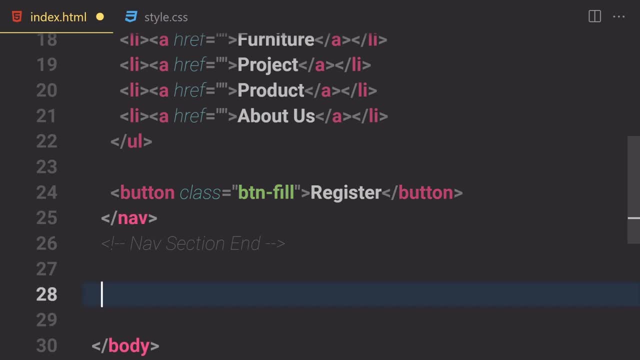 navigation as well. so now section end- navigation as well. so now section end. so now let's just get into our html. and so now let's just get into our html. and so now let's just get into our html and start working on our header area so that 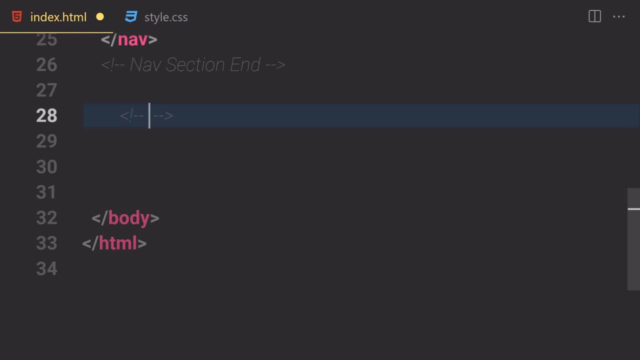 start working on our header area. so that start working on our header area. so that was just a coding for navigation. so now was just a coding for navigation. so now was just a coding for navigation. so now let's just start working on our header. let's just start working on our header. 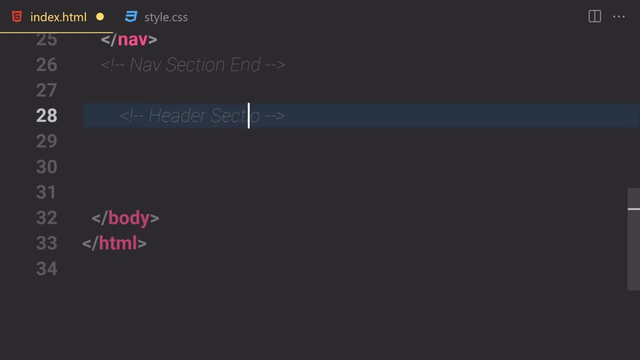 let's just start working on our header area. so i'm going to write a comment for area. so i'm going to write a comment for area. so i'm going to write a comment for myself. like a header- uh section. start myself like a header- uh section- start. 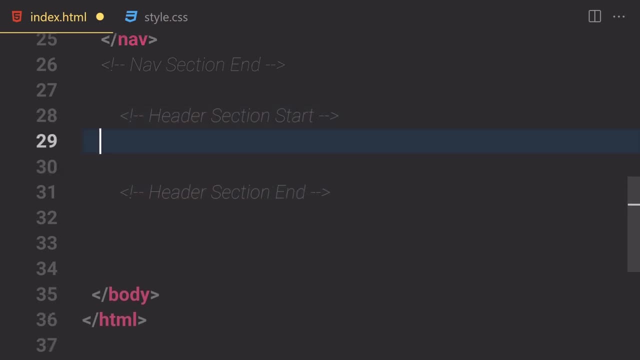 myself like a header uh section. start and duplicate that, and this is going to and duplicate that, and this is going to and duplicate that, and this is going to be the end of that header section. so be the end of that header section. so be the end of that header section. so what do we have to do? first of all, we 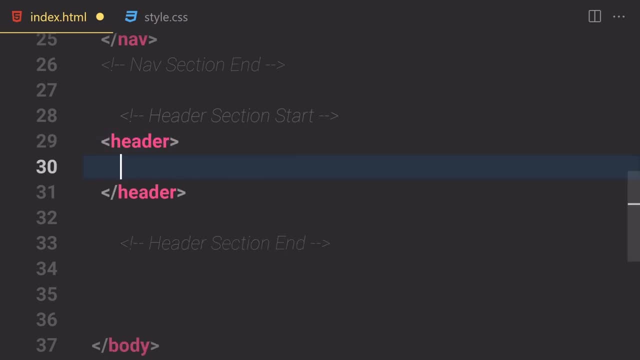 what do we have to do first of all? we? what do we have to do first of all? we are going to be writing a header and are going to be writing a header, and are going to be writing a header, and we're not going to be giving any classes. 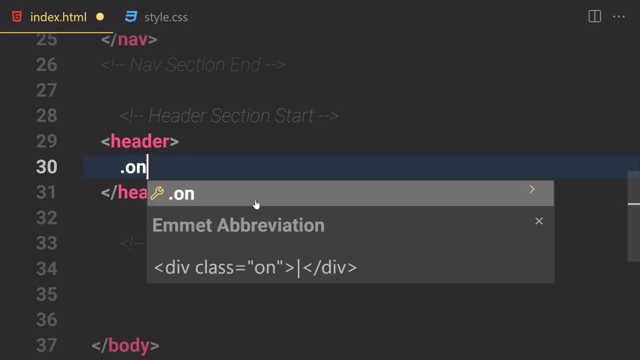 we're not going to be giving any classes, we're not going to be giving any classes, and whatsoever. so then we have to create and whatsoever. so then we have to create, and whatsoever. so then we have to create a content, a content, a content, content and then container. so, inside this, content and then container. so inside this content and then container. so inside this content container, we are going to be content container. we are going to be content container. we are going to be writing h1 with the class of main, writing h1 with the class of main. 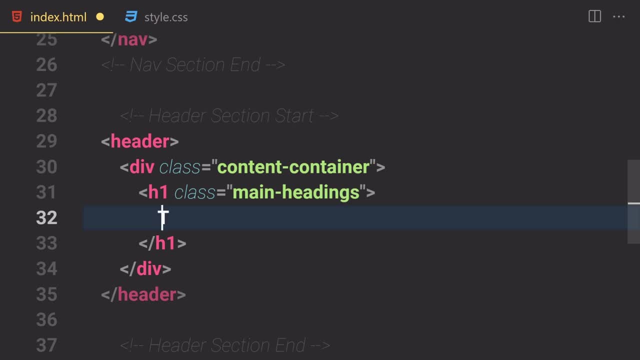 writing h1 with the class of main headings. so these are going to be the headings, so these are going to be the headings, so these are going to be the main headings of our main headings, of our main headings of our webpage. so the most, and then br. 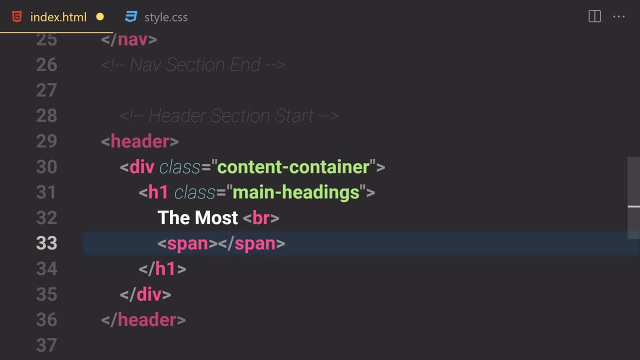 headings of our webpage- so the most. and then br- headings of our webpage, so the most, and then br. and now let's just provide like span in, and now let's just provide like span in, and now let's just provide like span in here, and we're not going to be giving. 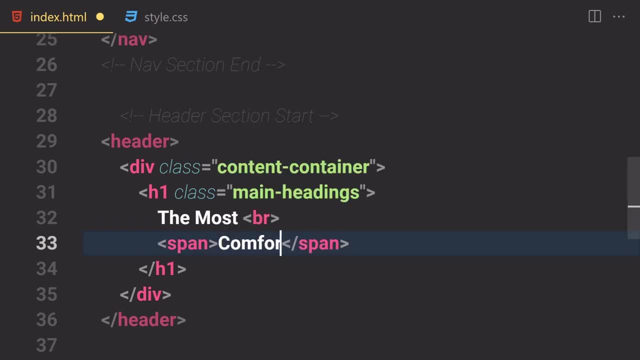 here and we're not going to be giving here, and we're not going to be giving any classes whatsoever so comfortable, any classes whatsoever so comfortable, any classes whatsoever so comfortable from fur table, from fur table, from fur table. okay, and also provide a br in here, and 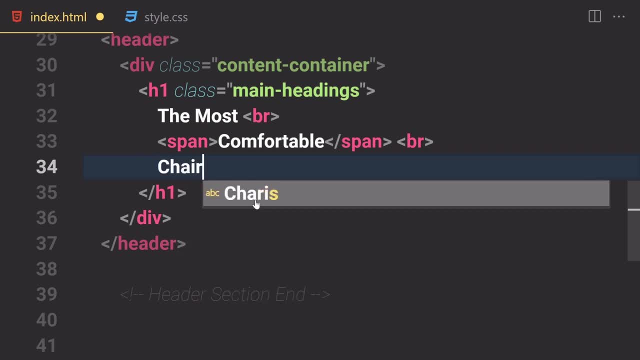 okay, and also provide a br in here. and okay, and also provide a br in here, and now, let's just start working. or you, now, let's just start working. or you, now, let's just start working. or you know i'm gonna write like a chair. know i'm gonna write like a chair. 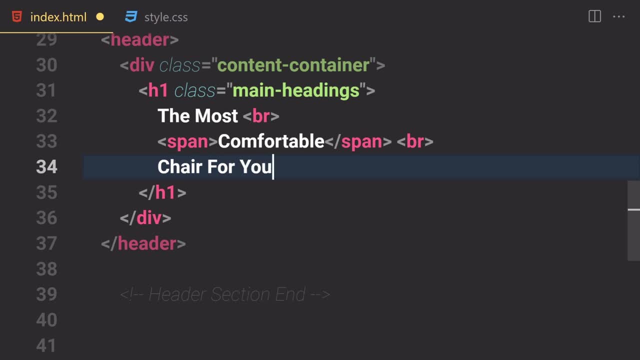 know i'm gonna write like a chair for you, for you, for you, or you in a capitalized cases and now, or you in a capitalized cases and now, or you in a capitalized cases, and now, underneath this h1, underneath this h1, underneath this h1, what do we have to do? we are going to be. 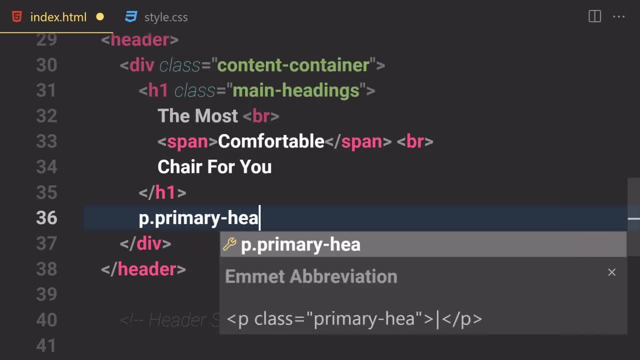 what do we have to do? we are going to be. what do we have to do? we are going to be writing a p with a class of writing a p with a class of writing a p with a class of primary headings. okay, so inside there. primary headings- okay, so inside there. primary headings. okay, so inside there, i'm going to put a lorem ipsum, just like i'm going to put a lorem ipsum, just like i'm going to put a lorem ipsum, just like. so, oh, you know what i'm going to. so, oh, you know what i'm going to. 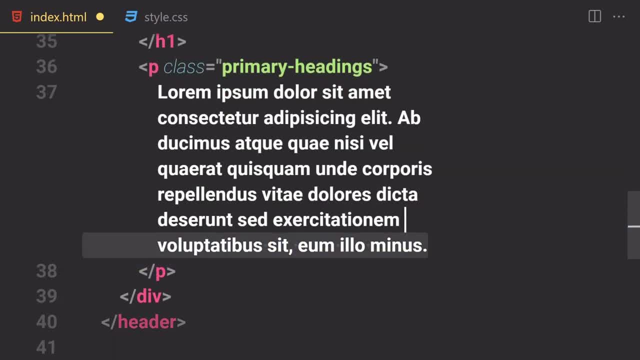 so, oh, you know what i'm going to remove that, remove that, remove that. oh my goodness, i didn't mean to do that. oh my goodness, i didn't mean to do that. oh my goodness, i didn't mean to do that. let's just remove these, uh, two lines from. 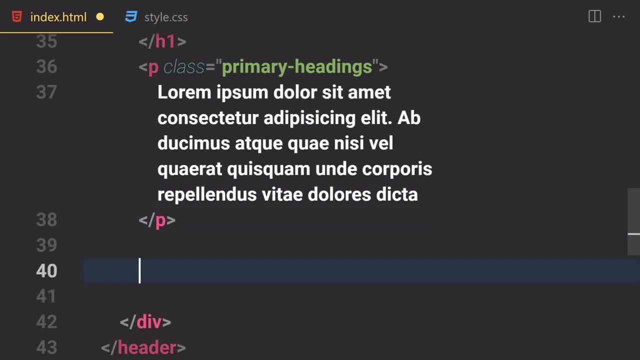 let's just remove these uh two lines from. let's just remove these uh two lines from there and underneath this paragraph, there and underneath this paragraph, there and underneath this paragraph tag. we have to create a buttons container tag. we have to create a buttons container tag. we have to create a buttons container so that we can reuse that again. and 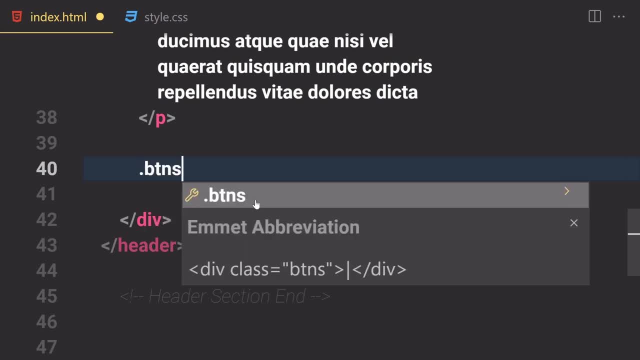 so that we can reuse that again, and so that we can reuse that again and again. so now let's just use again. so now let's just use again. so now let's just use what btn or you know btns would be fine, what btn or you know btns would be fine. 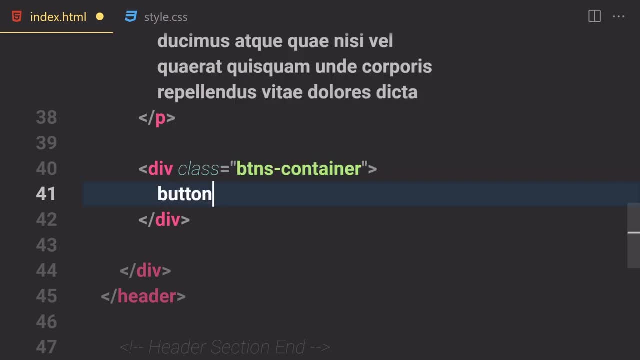 what btn or you know btns would be fine in container inside there. we are going in container inside there. we are going in container inside there. we are going to be creating two buttons with the. to be creating two buttons with the. to be creating two buttons with the class of btn fill. so it will just fill. 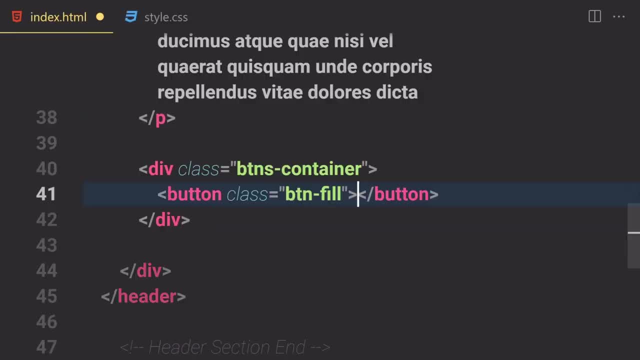 class of btn fill, so it will just fill class of btn fill. so it will just fill that button and it will take the that button and it will take the that button and it will take the styling which we just put right here. so styling which we just put right here, so 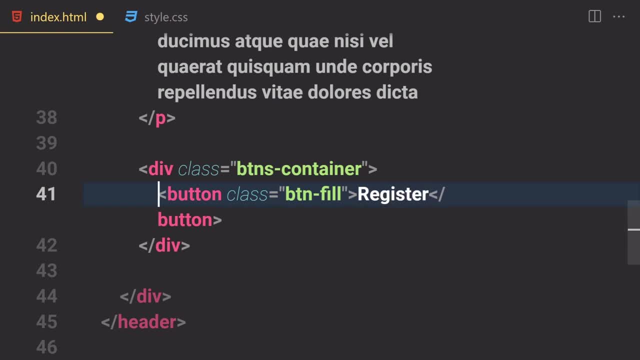 styling which we just put right here. so now let's just write like a register. now let's just write like a register. now let's just write like a register, and now let's just start working on our. and now let's just start working on our, and now let's just start working on our new button. so let's just create that and 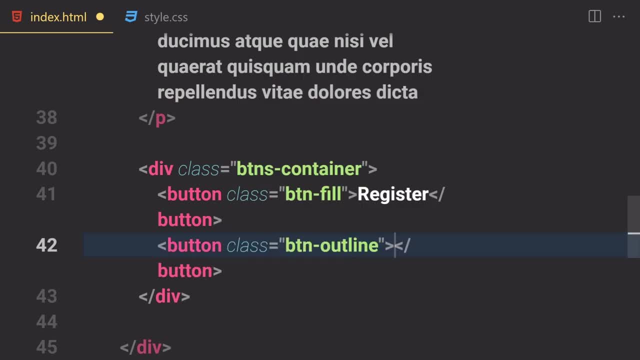 new button, so let's just create that. and new button, so let's just create that. and this is going to be it for the btn. this is going to be it for the btn. this is going to be it for the btn: outline so outline so outline. so it will just say, like: learn more, i want. 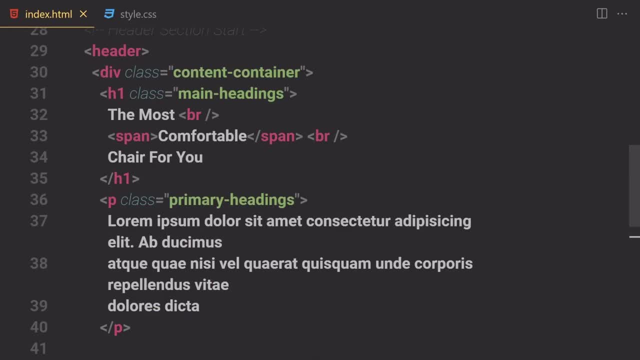 it will just say like: learn more, i want. it will just say: like: learn more, i want to just zoom out a bit, and this is how to just zoom out a bit. and this is how to just zoom out a bit and this is how it looks like. so, if you sell a file, so 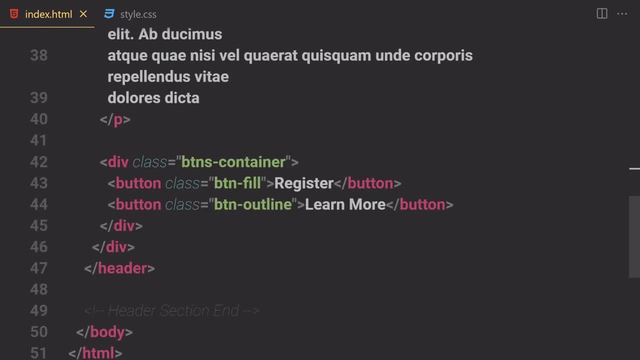 it looks like so if you sell a file. so it looks like so if you sell a file. so these are the html coding for header. these are the html coding for header. these are the html coding for header area. all right, so now let's just get in. 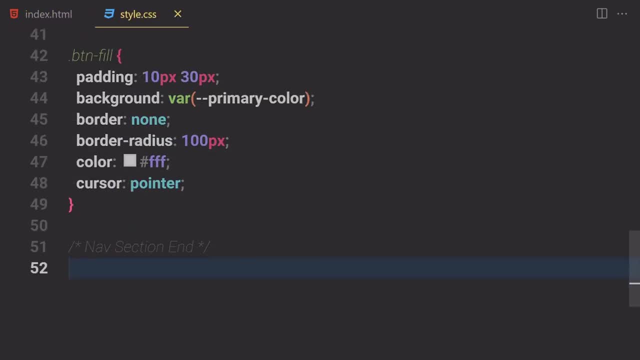 area all right, so now let's just get in area. all right, so now let's just get in towards css. and now let's just style towards css. and now let's just style towards css. and now let's just style that a bit, that a bit, that a bit. all right. so here what i'm going to do: 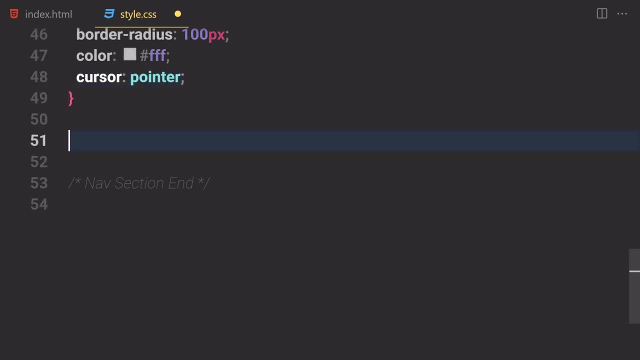 all right, so here what i'm going to do. all right, so here, what i'm going to do is that i'm going to first of all start. is that i'm going to first of all start. is that i'm going to first of all start from that button. so, 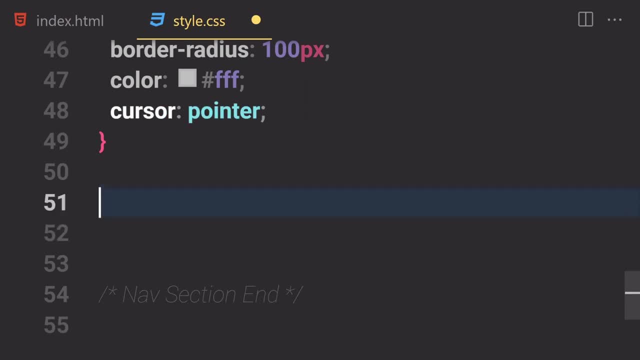 from that button, so from that button, so so that we can put our buttons in one, so that we can put our buttons in one, so that we can put our buttons in one place. so you know, i'm going to just place. so you know, i'm going to just. 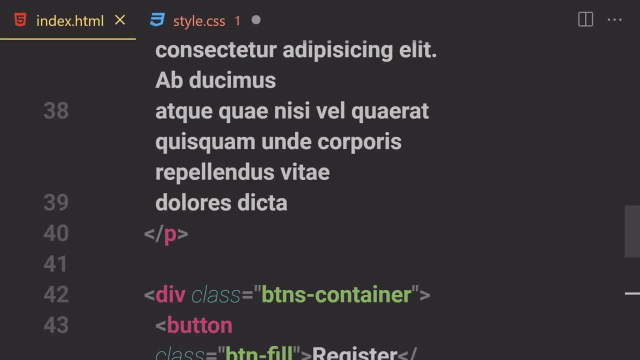 place. so you know, i'm going to just start working on our btn and outline so place. so you know, i'm going to just start working on our btn and outline so which is the button which we create, which is the button which we create, which is the button which we create right here. so this btn outline, all right. 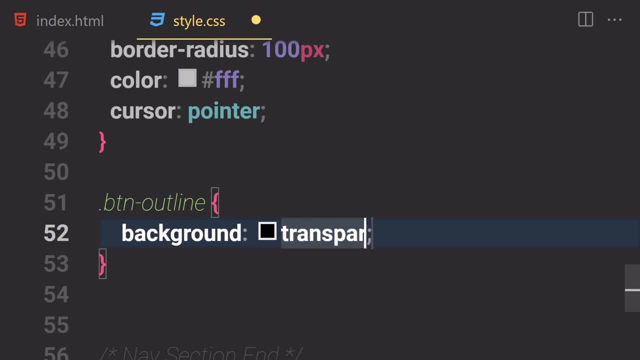 right here. so this btn outline all right, right here, so this btn outline all right, so, so, so i'm going to provide a background color, i'm going to provide a background color. i'm going to provide a background color to be totally transparent because we, to be totally transparent because we. 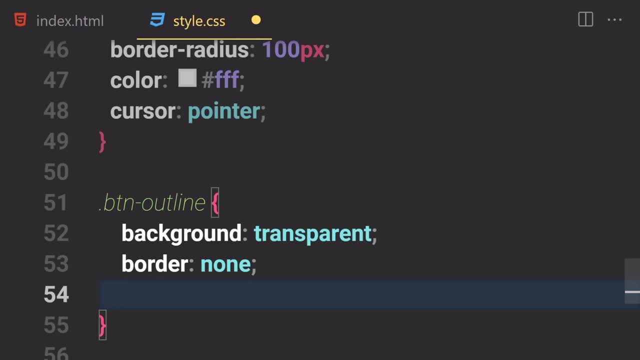 to be totally transparent, because we want to remove that background and also want to remove that background and also want to remove that background and also that border. okay, so i'm going to just that border okay, so i'm going to just that border okay. so i'm going to just give margin for the left, like 20 pixel. 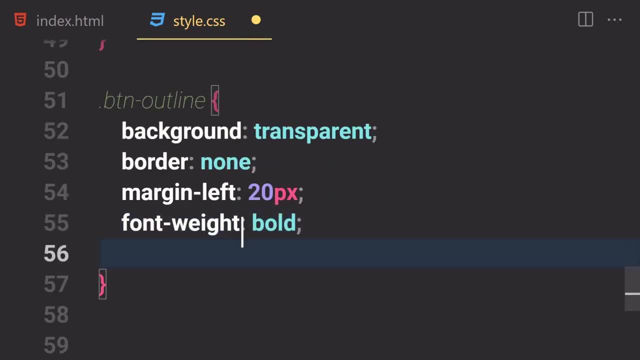 give margin for the left like 20 pixel. give margin for the left like 20 pixel. and now let's just increase the font. and now let's just increase the font, and now let's just increase the font. weight of that or not increase. but weight of that or not increase. but 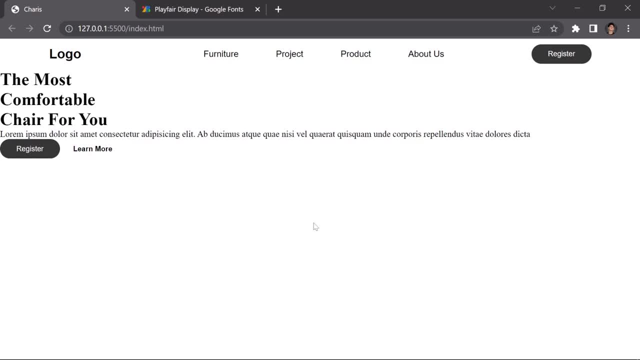 weight of that or not increase. but uh, just probably a bit of boldness to it. uh, just probably a bit of boldness to it. uh, just probably a bit of boldness to it. so a cursor will be pointer if you save. so a cursor will be pointer if you save. 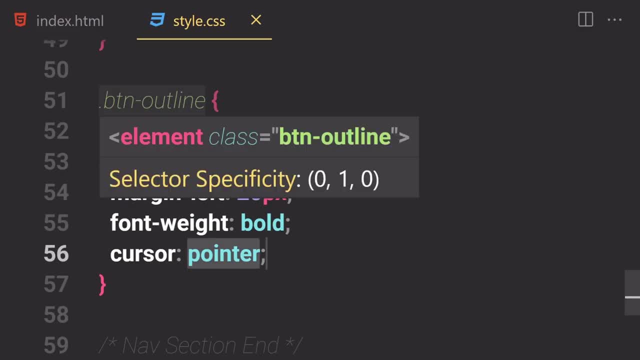 so a cursor will be pointer if you save that and this is how it looks like for that and this is how it looks like for that and this is how it looks like for now. okay, so just actual tech now. okay. so just actual tech now. okay. so just actual tech, tech text to be precise, not tech. uh, you. 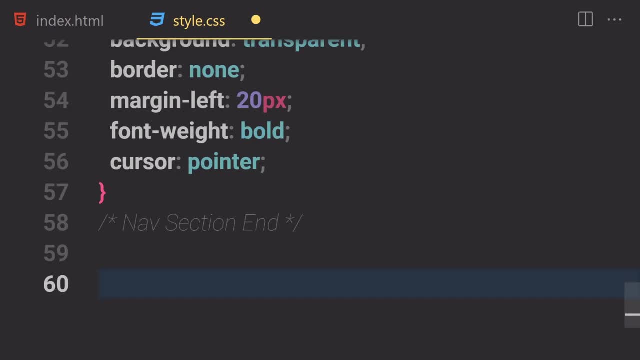 tech text, to be precise, not tech. uh, you tech text, to be precise, not tech. uh, you know what i'm gonna put it right here. know what i'm gonna put it right here. know what i'm gonna put it right here. so now let's just create a new comment. 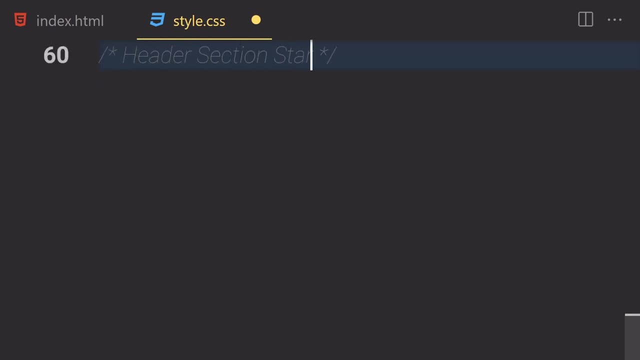 so now, let's just create a new comment. so now, let's just create a new comment for myself, like a header section start for myself. like a header section start for myself, like a header section start, and i'm going to just zoom out a bit so, and i'm going to just zoom out a bit so. and i'm going to just zoom out a bit so you guys can see everything a bit better. you guys can see everything a bit better. you guys can see everything a bit better, and we are going to start working on our. and we are going to start working on our. 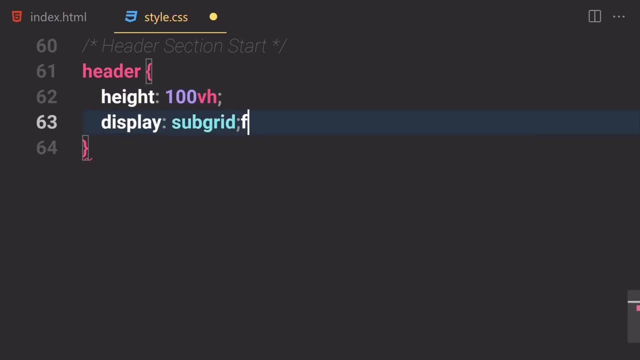 and we are going to start working on our headers. so i'm going to give a height of headers. so i'm going to give a height of headers. so i'm going to give a height of like 100 vh display will be now set to. like 100 vh display will be now set to. 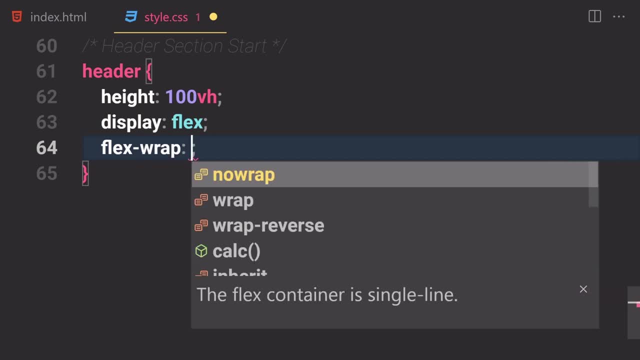 like 100 vh display will be now set to totally flex, because you want them to be totally flex, because you want them to be totally flex, because you want them to be like totally flexible and flex wrap will like totally flexible and flex wrap will like totally flexible and flex wrap will be now set to wrap. 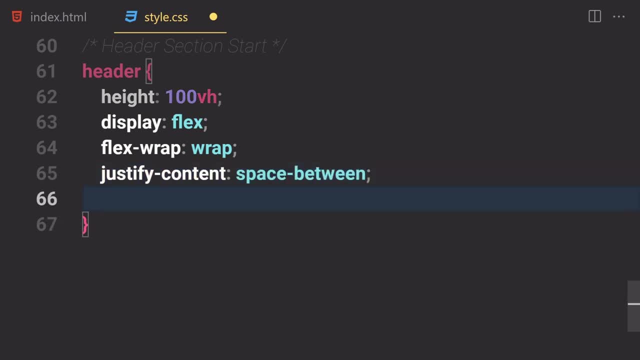 be now set to wrap. be now set to wrap and justify content. i'm going to set and justify content. i'm going to set and justify content. i'm going to set that to like space between: in this case. that to like space between: in this case. that to like space between: in this case, and align. items will be now set to. 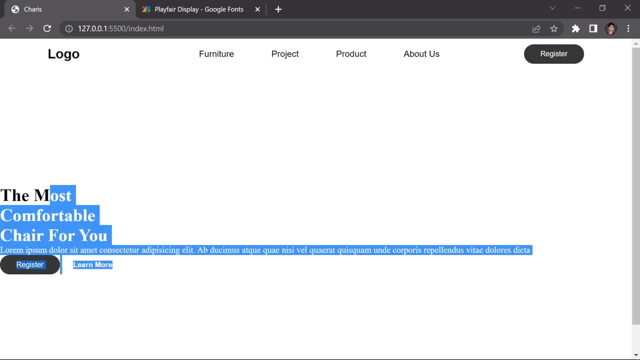 and align items will be now set to: and align items will be now set to: totally centered. so if you save that and totally centered, so if you save that and totally centered, so if you save that, and this is how currently things looks like, this is how currently things looks like. 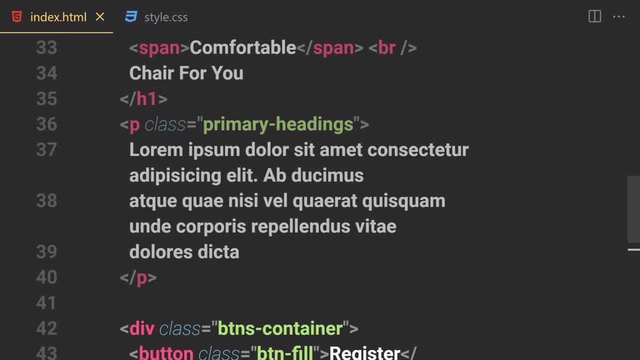 this is how currently things looks like. all right, so what else do we have to do? all right, so what else do we have to do? all right, so what else do we have to do? we have to select that content container. we have to select that content container. 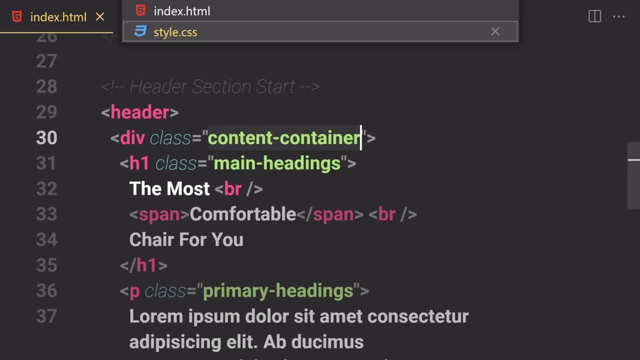 we have to select that content container. which is which is? which is on this content container right here. so on this content container right here. so on this content container, right here. so i'm going to just copy that, i'm going to just copy that, i'm going to just copy that and i'm going to select it right here. so 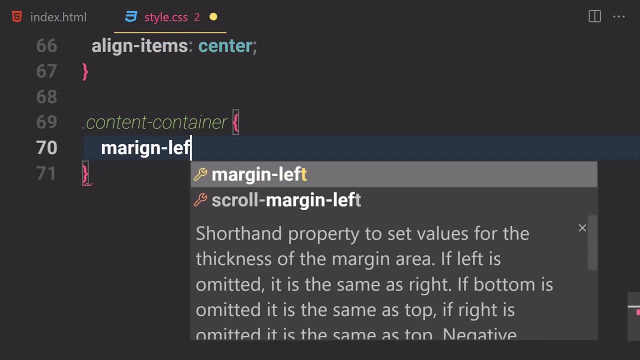 and i'm going to select it right here. so, and i'm going to select it right here, so i'm going to paste it, i'm going to paste it, i'm going to paste it, and let's just point a margin for the. and let's just point a margin for the. 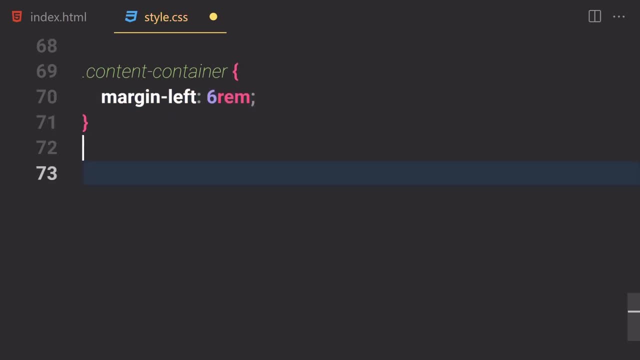 and let's just point a margin for the left to be like six rims, and also let's left to be like six rims, and also let's left to be like six rims, and also let's just start working on our headings. so, just start working on our headings. so. 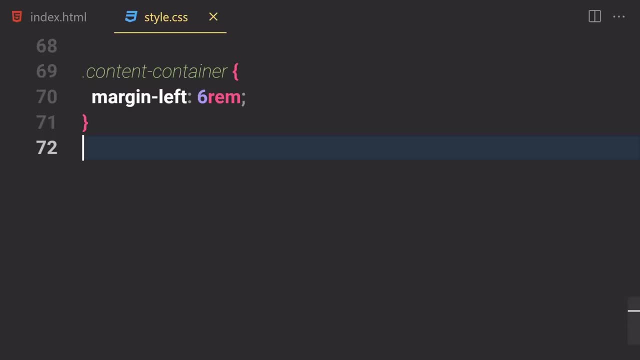 just start working on our headings, so these headings, so i'm going to just these headings, so i'm going to just these headings, so i'm going to just make that a little bit bigger and stuff, make that a little bit bigger and stuff, make that a little bit bigger and stuff. so the class was like main heading i'm. so the class was like main heading i'm. so the class was like main heading. i'm going to copy that real quick, going to copy that real quick, going to copy that real quick and i'm going to just space it right and i'm going to just space it right. 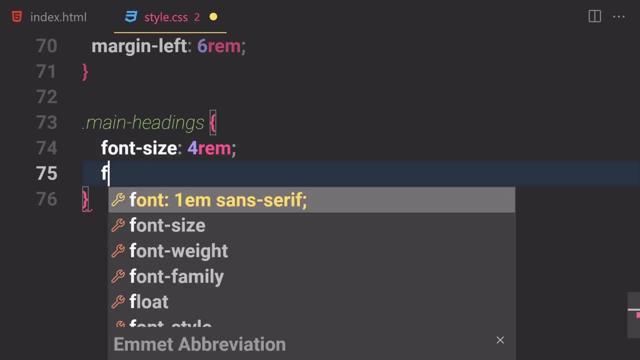 and i'm going to just space it right there. so i'm going to just write a font there. so i'm going to just write a font there. so i'm going to just write a font size of like four ram on family. i'm size of like four ram on family. i'm. 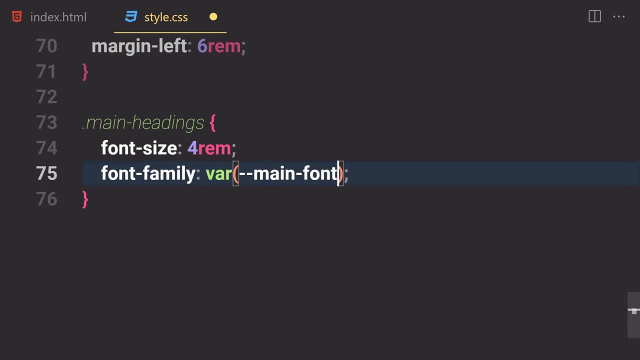 size of, like four ram on family. i'm going to change that to like, going to change that to like, going to change that to like one of main form, so which we declare one of main form, so which we declare one of main form, so which we declare above and color, in this case, is going. 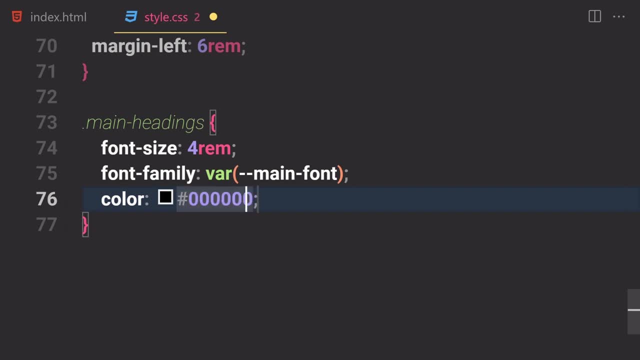 above and color in this case is going above and color in this case is going to be like uh one, two, three. to be like uh one, two, three. to be like uh one, two, three and four, five, six and four and four, five, six and four and four, five, six and four f. okay, so this kind of a bluish. 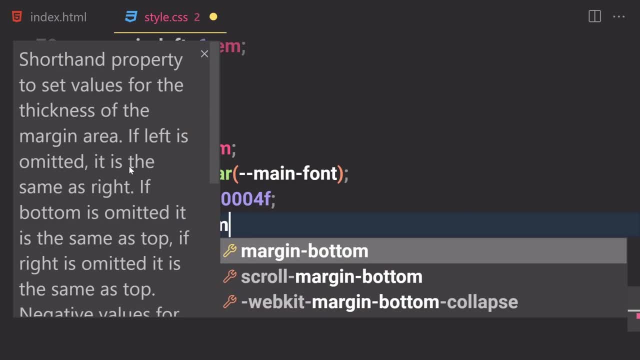 f. okay. so this kind of a bluish f? okay. so this kind of a bluish black color, whatever you want to call black color, whatever you want to call black color, whatever you want to call it, and then we have margin for a bottom it, and then we have margin for a bottom. 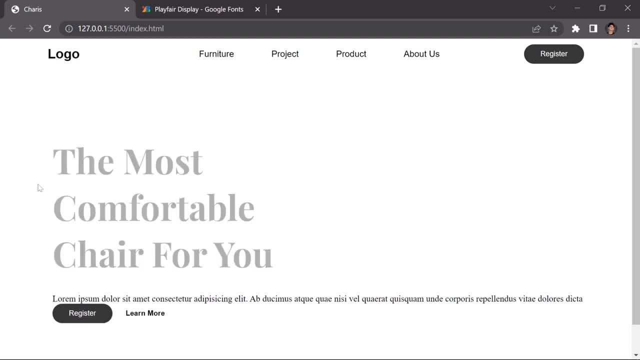 it, and then we have margin for a bottom of two rims. so if you sell that of two rims, so if you sell that of two rims, so if you sell that- and this is how it looks like right here. and this is how it looks like right here. 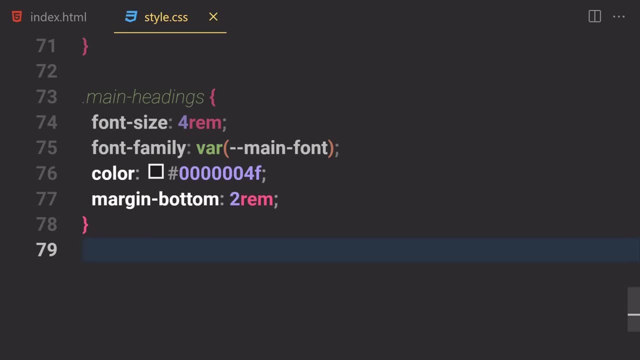 and this is how it looks like right here now. i'm going to just take care of that now. i'm going to just take care of that now. i'm going to just take care of that and i want to make that to like totally, and i want to make that to like totally. 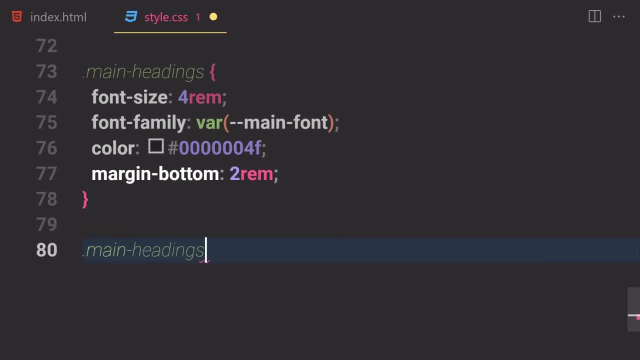 and i want to make that to like totally pure black colored. so i'm going to just pure black colored. so i'm going to just pure black colored. so i'm going to just write like our main headings and now write like our main headings. and now write like our main headings and now inside this main headings we have a span. inside this main headings, we have a span. inside this main headings, we have a span. let me just show you that real quick. so let me just show you that real quick. so let me just show you that real quick. so now we want to select that one and we 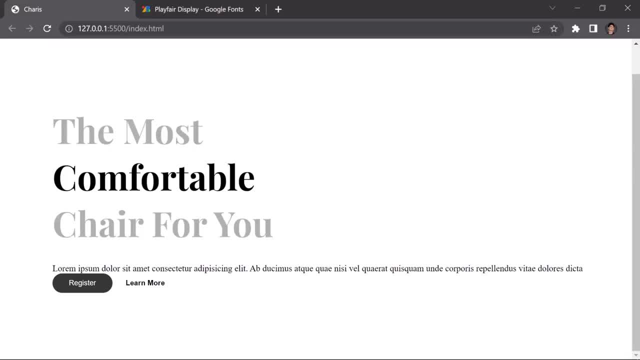 now we want to select that one and we now we want to select that one and we want to just provide a totally black, want to just provide a totally black, want to just provide a totally black color on it. so if you sell that and boom color on it. so if you sell that and boom, color on it. so if you sell that and boom, this is how it looks like, all right. so this is how it looks like, all right. so this is how it looks like, all right. so now, let's just take care of these. now, let's just take care of these. 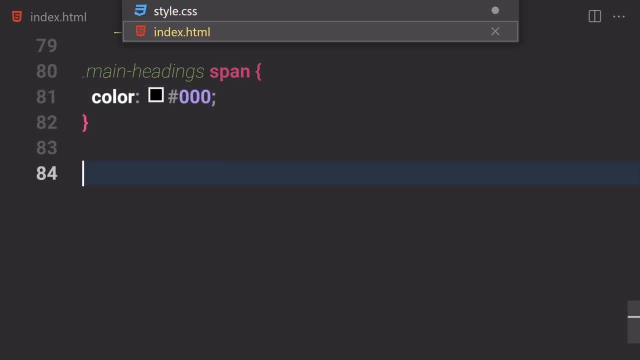 now let's just take care of these primary headings. real quick. primary headings, real quick. primary headings, real quick. so i'm going to just select that from. so i'm going to just select that from. so i'm going to just select that from here. i'm going to write copy there to. 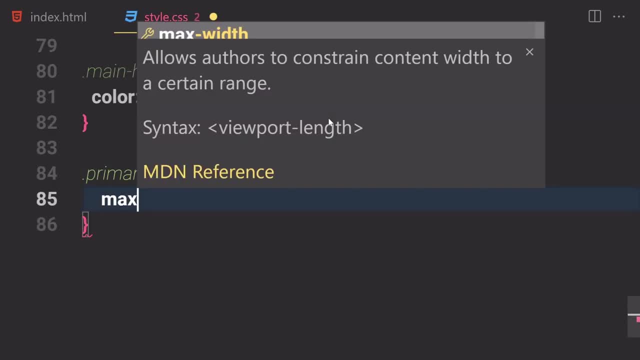 here i'm going to write copy there to. here i'm going to write copy there to be precise, not right. and let's just be precise, not right. and let's just be precise, not right, and let's just provide a max. provide a max, provide a max. uh, width will be like i don't know, 500. 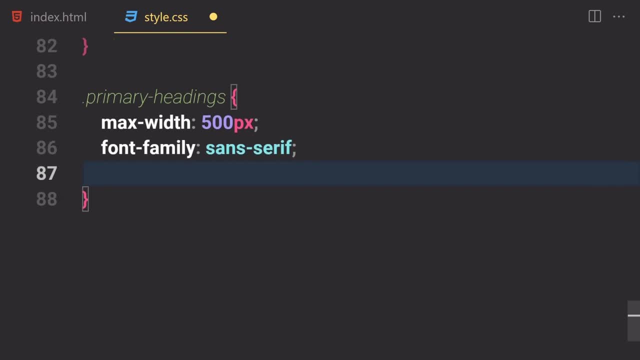 uh width will be like i don't know. 500 uh width will be like i don't know. 500 pixel will be fine and font family will. pixel will be fine and font family will. pixel will be fine and font family will be also set to send surf and line height. 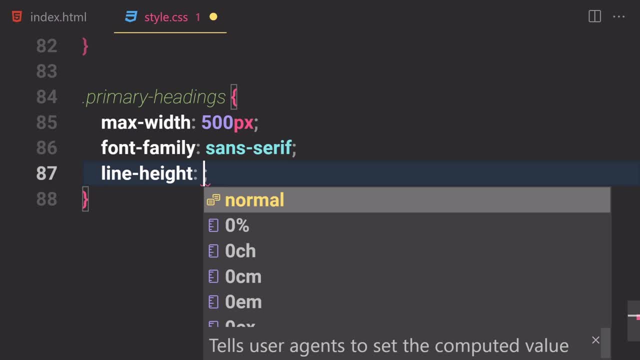 be also set to send surf and line height be also set to send surf and line height. i'm going to just provide a little bit. i'm going to just provide a little bit. i'm going to just provide a little bit of line, of line of line height to it, like i don't know: 25 pixel. 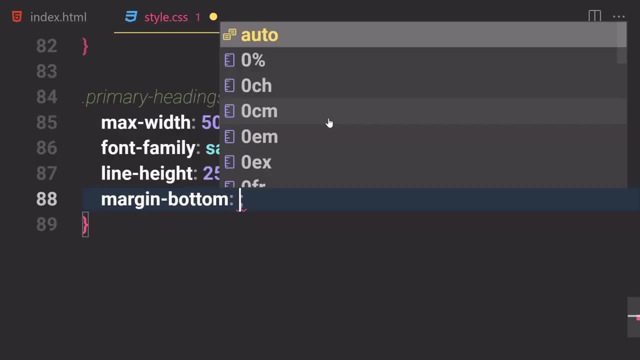 height to it, like i don't know, 25 pixel height to it, like i don't know. 25 pixel will be fine and margin for the bottom will be fine and margin for the bottom will be fine and margin for the bottom i'm going to give it like two rim and 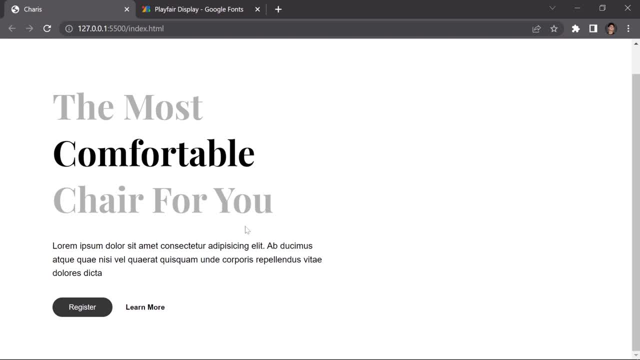 i'm going to give it like two rim, and i'm going to give it like two rim, and now, if you save that, and this is how it now, if you save that, and this is how it now, if you save that, and this is how it looks like for now, anyway, so it's. 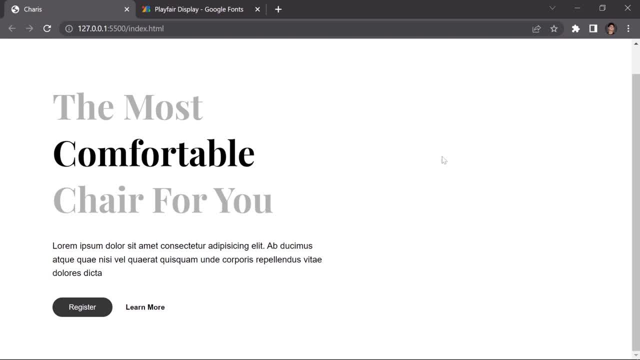 looks like for now anyway. so it's looks like for now anyway. so it's looking better now. let's just take care looking better now. let's just take care looking better now. let's just take care of that image container first of all. so, of that image container first of all, so. 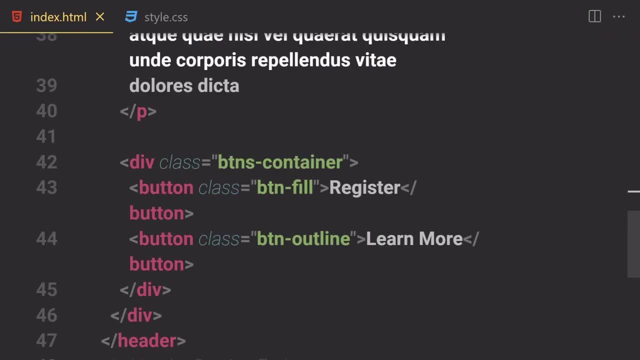 of that image container first of all. so we have to write html code for that. so we have to write html code for that. so we have to write html code for that. so let me just get into it and underneath. let me just get into it and underneath. 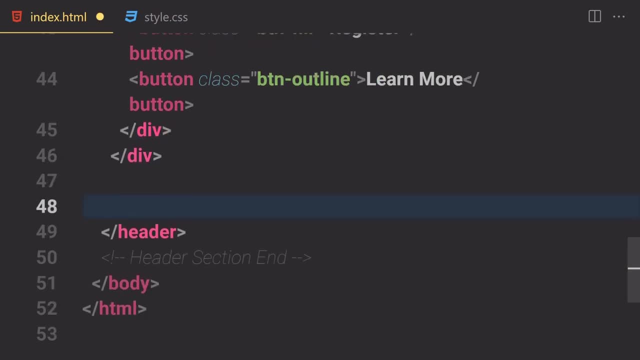 let me just get into it. and underneath everything so underneath this div and everything so underneath this div and everything so underneath this div and stuff so inside a header area, but stuff so inside a header area, but stuff so inside a header area, but underneath these buttons and all of their. 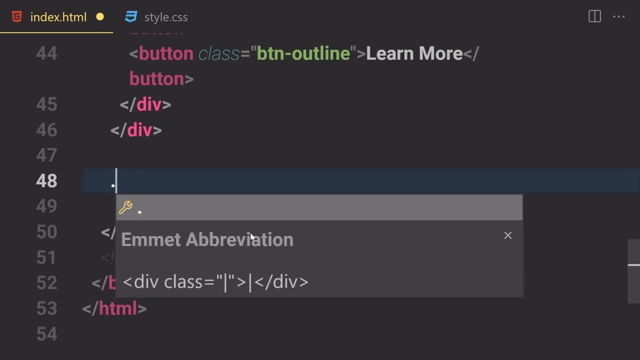 underneath these buttons and all of their, underneath these buttons and all of their containers. so we have to create containers. so we have to create containers. so we have to create another div with the class of img, and then another div with the class of img, and then another div with the class of img, and then container, uh, container, like so. 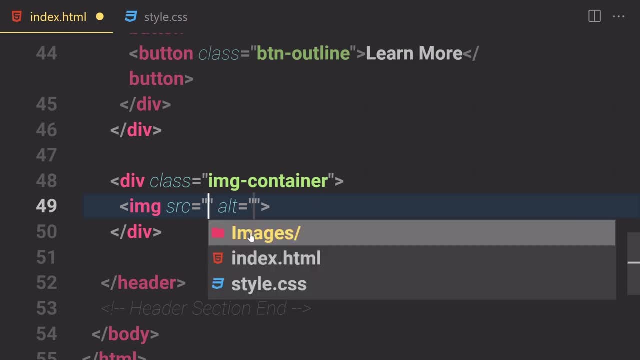 container, uh, container like so. container, uh, container like so, and let's just render our image. so let's, and let's just render our image, so let's, and let's just render our image. so let's just go to our images somewhere. so i'm just go to our images somewhere, so i'm. 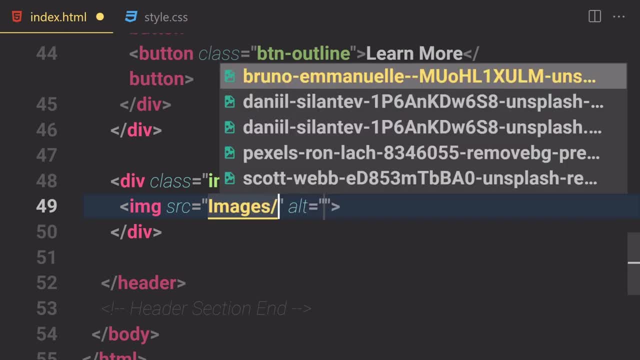 just go to our images somewhere. so i'm going to hit control space, select this. going to hit control space, select this. going to hit control space, select this- images folder. and i'm going to just images folder and i'm going to just images folder and i'm going to just select that, daniel or 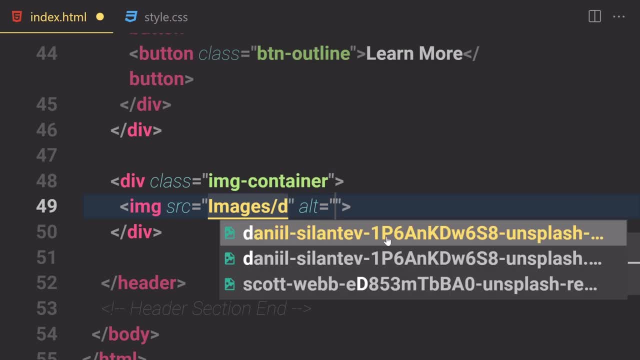 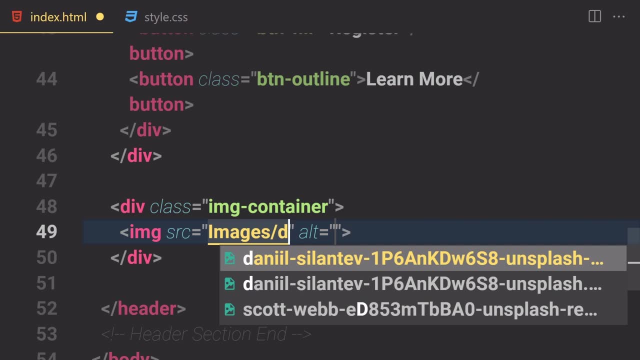 select that daniel, or select that daniel, or, uh, i guess, which one should i choose? uh, okay, i'm going to zoom out a bit. first of all, let's just zoom out a bit. i'm going to zoom out a bit. first of all, let's just zoom out a bit. 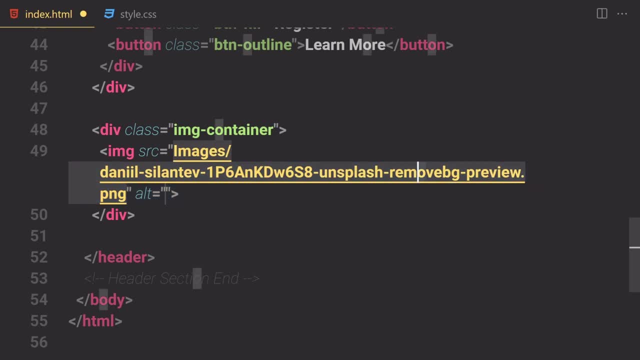 i'm going to zoom out a bit. so you know, i'm going to select this one. so you know i'm going to select this one. so you know i'm going to select this one and remove bg1. so i'm going to just and remove bg1. so i'm going to just. 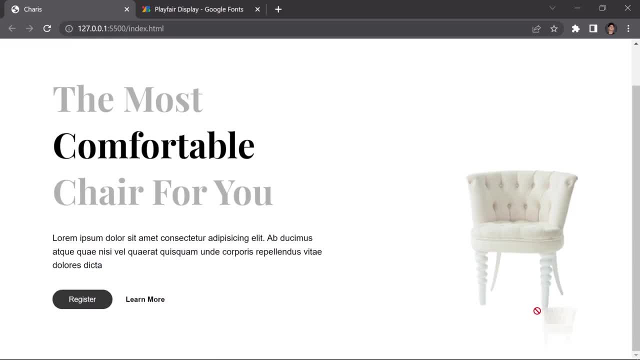 and remove bg1. so i'm going to just select this, remove bg. and now, if you select this, remove bg. and now, if you select this, remove bg. and now, if you save a file server log. uses this image: save a file server log. uses this image: save a file server log. uses this image: right here. 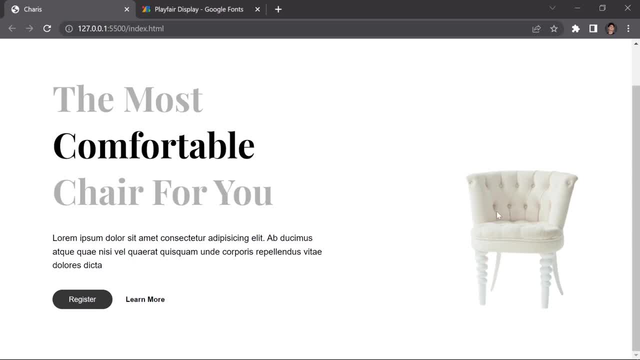 right here, right here, with the background removed. so i've with the background removed, so i've with the background removed, so i've already removed the background from, already removed the background from, already removed the background from this image. so that's why we can see this image, so that's why we can see. 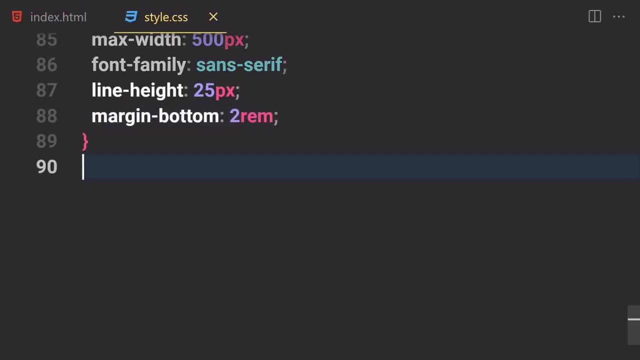 this image. so that's why we can see that that that without any background and stuff. so now without any background and stuff. so now without any background and stuff. so now let's just get into our css, and now let's just get into our css. and now 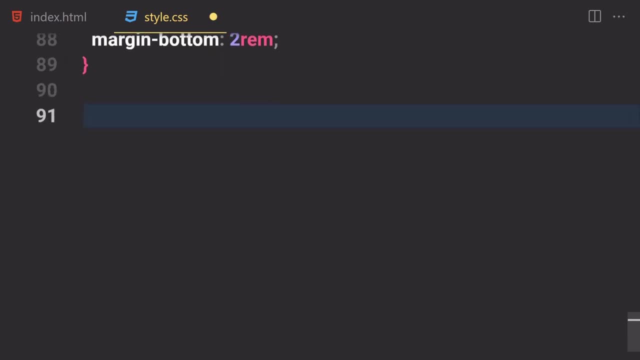 let's just get into our css and now, let's just style that a bit, let's just style that a bit, let's just style that a bit. so what i'm going to do? so, what i'm going to do. so, what i'm going to do, first of all, let me just select my img. 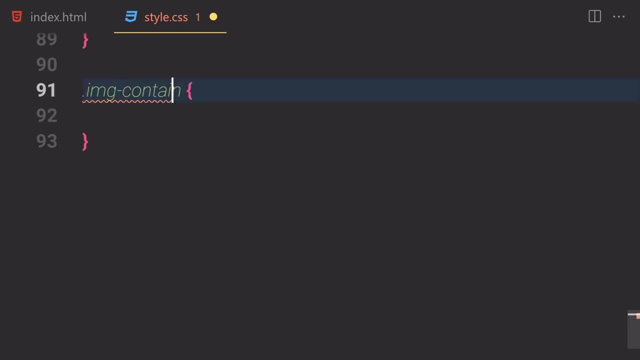 first of all, let me just select my img. first of all let me just select my img and container, so con and container, so con and container, so con tiner, like so which is this class like img tiner like so which is this class like img tiner like so which is this class like img container? i want to copy it from here. 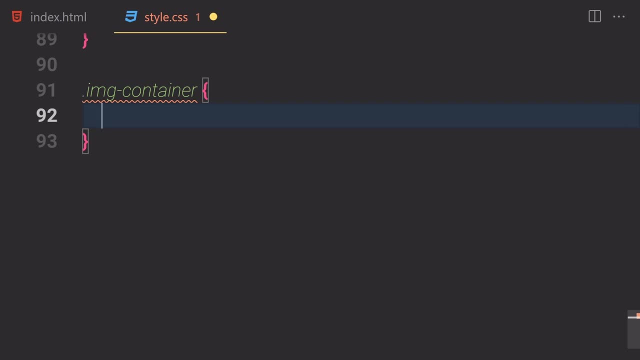 container- i want to copy it from here. container- i want to copy it from here. i'm going to paste it right here. so i i'm going to paste it right here, so i i'm going to paste it right here. so i want to make sure that we select the 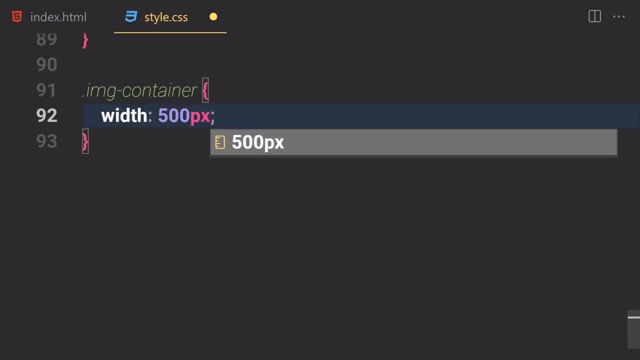 want to make sure that we select the want to make sure that we select the same div. so let's just provide a width, same div. so let's just provide a width, same div. so let's just provide a width of like 500 pixel, and i'm going to of like 500 pixel and i'm going to of like 500 pixel and i'm going to duplicate, then i'm going to change that duplicate, then i'm going to change that duplicate, then i'm going to change that to like height and let's just use a. 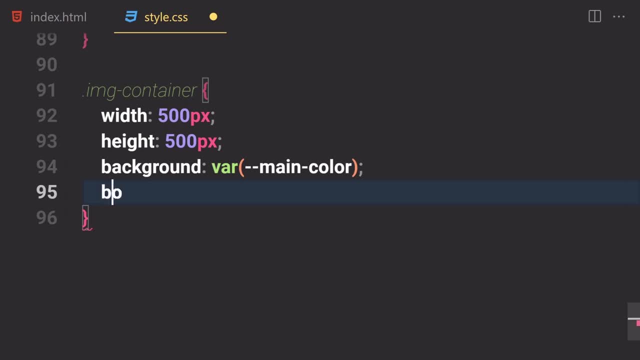 to like height, and let's just use a to like height and let's just use a background color to be like totally main background color, to be like totally main background color, to be like totally main color. okay, so i'm gonna also provide a color. okay, so i'm gonna also provide a. 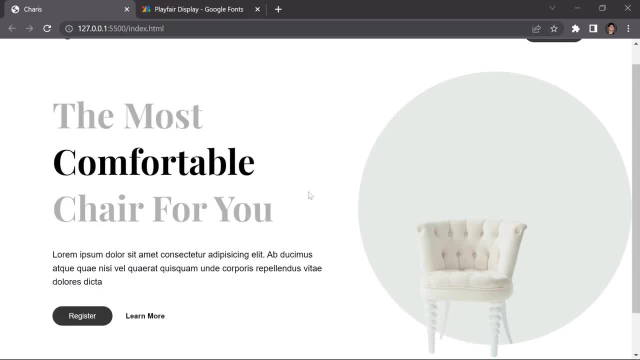 color. okay, so i'm gonna also provide a border radius to be like 100, border radius to be like 100, border radius to be like 100. and now, if you save that, so this is how. and now, if you save that, so this is how. and now, if you save that, so this is how it looks like right now. 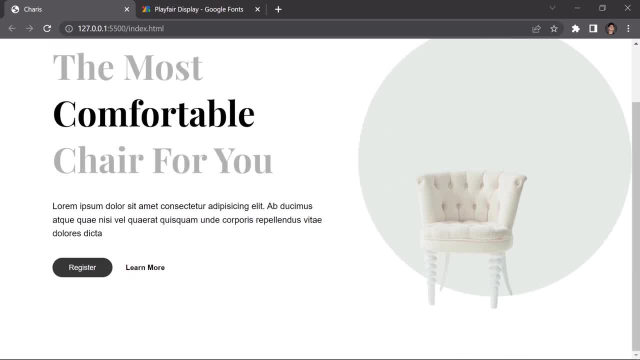 it looks like right now. it looks like right now, for now it's going to be like totally. for now it's going to be like totally. for now it's going to be like totally, totally unresponsive, like not responsive, totally unresponsive, like not responsive, totally unresponsive, like not responsive. so we can make that responsive once we. 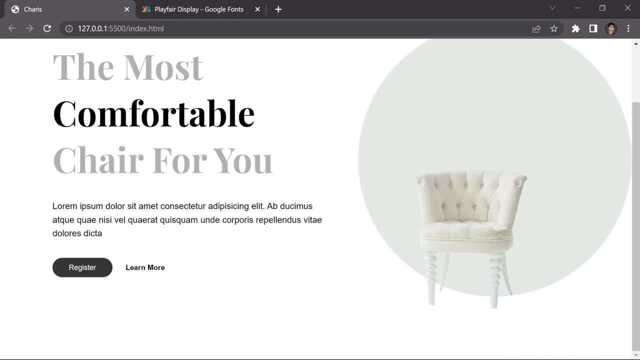 so we can make that responsive once we. so we can make that responsive once we jump into media queries. but you don't jump into media queries. but you don't jump into media queries but you don't have to worry about their responsiveness. have to worry about their responsiveness. 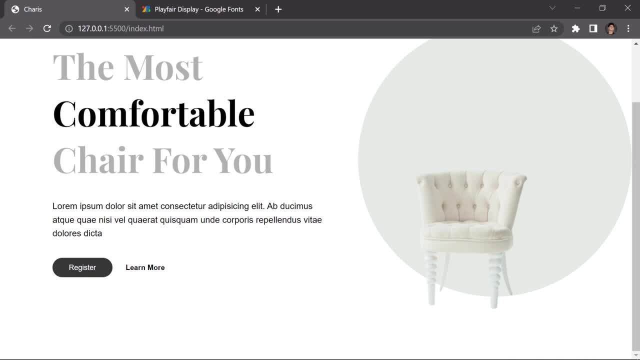 have to worry about their responsiveness and all of that stuff for now, so what? and all of that stuff for now, so what? and all of that stuff for now. so what else do we have to do? let's just take. else do we have to do? let's just take. 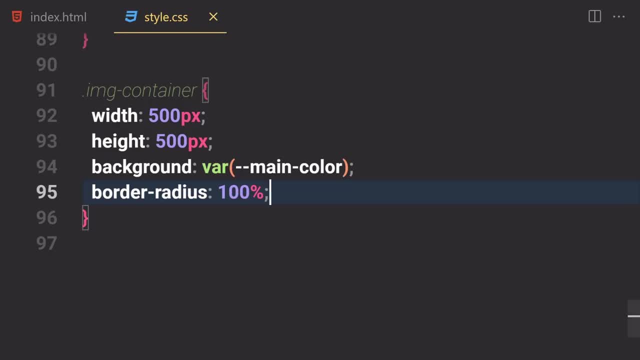 else do we have to do? let's just take care of that image, because it's looking care of that image, because it's looking care of that image, because it's looking a bit smaller, a bit smaller, a bit smaller, and let's just take care of that real. 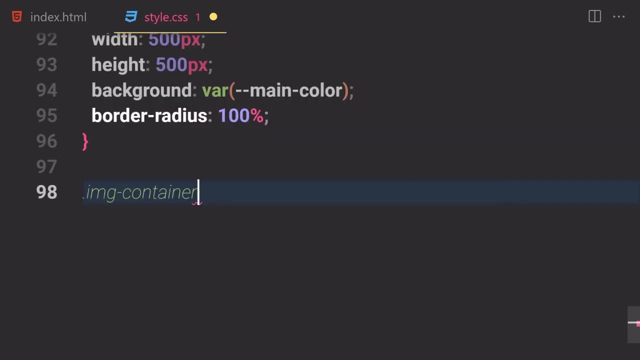 and let's just take care of that real. and let's just take care of that real, quick. so image container. so i'm going to quick, so image container, so i'm going to quick, so image container, so i'm going to select my image container and inside 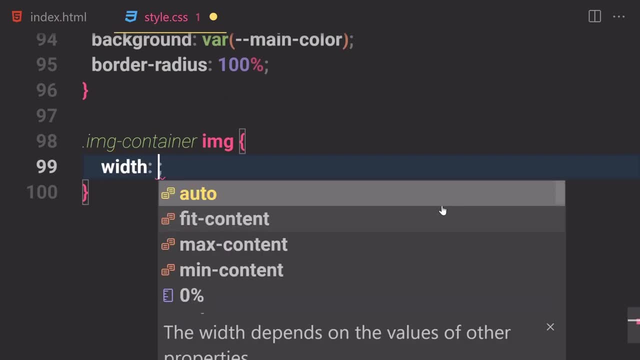 select my image container and inside, select my image container and inside this image container, i'm going to this image container, i'm going to this image container, i'm going to select that image and i'm going to just select that image and i'm going to select that image and i'm going to provide like a width of 400 pixel and 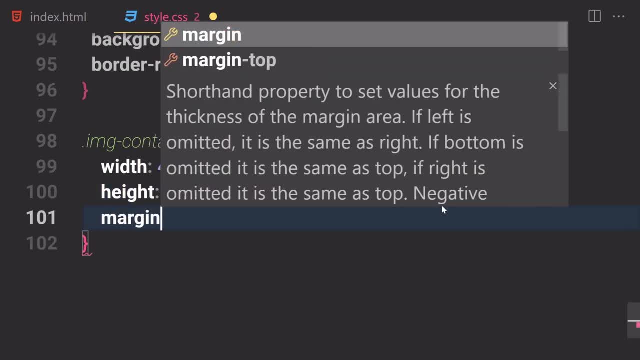 provide like a width of 400 pixel and provide like a width of 400 pixel and height will be 500 pixel and the margin height will be 500 pixel and the margin height will be 500 pixel and the margin for the left will be just 20 pixel. and. 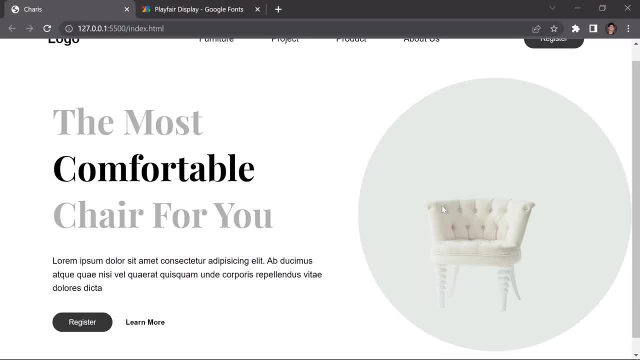 for the left will be just 20 pixel and for the left will be just 20 pixel and margin for the bottom will be 40 pixels. margin for the bottom will be 40 pixels. margin for the bottom will be 40 pixels. so now, if you save a file and this is: so now, if you save a file- and this is so now, if you save a file, and this is how it looks like for now. okay, so it's how it looks like for now. okay, so it's how it looks like for now. okay, so it's looking better. 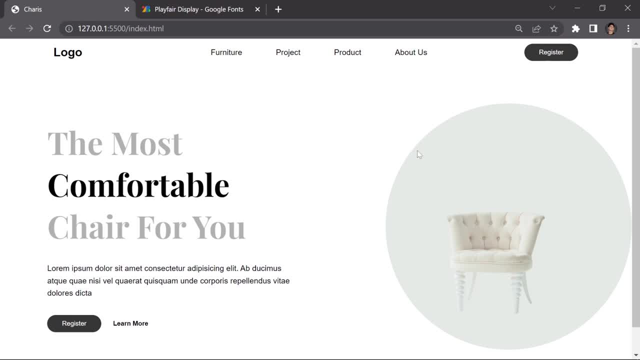 looking better, looking better, like so, like, so, like, so, anyways, so that's looking cool. if you, anyways, so that's looking cool. if you, anyways, so that's looking cool. if you want to change that around, so feel free. want to change that around, so feel free. want to change that around, so feel free to do that. so what else do we have to do? 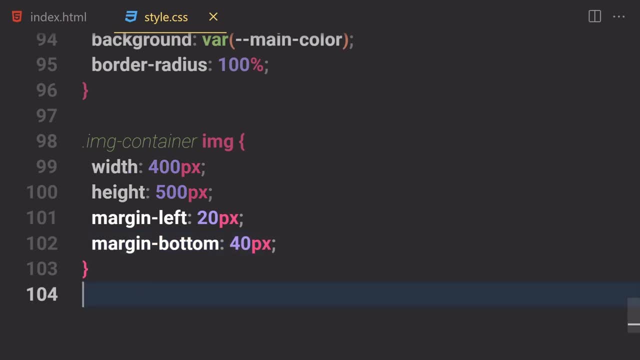 to do that. so what else do we have to do to do that? so what else do we have to do? let's just start working on our. let's just start working on our. let's just start working on our popularity section. so i'm going to write. 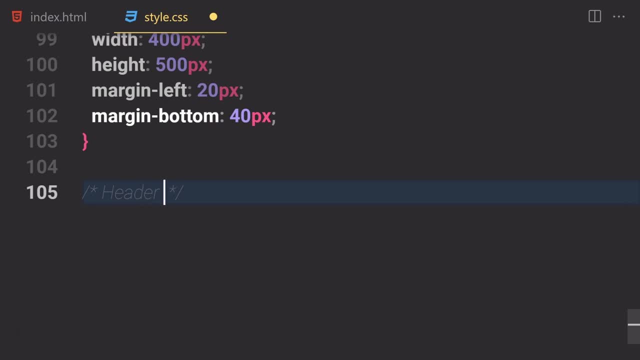 popularity section. so i'm going to write popularity section. so i'm going to write a comment for myself, like um a comment for myself, like um a comment for myself, like um, header, header, header, section. and hey, so now let's just get section and hey, so now let's just get. 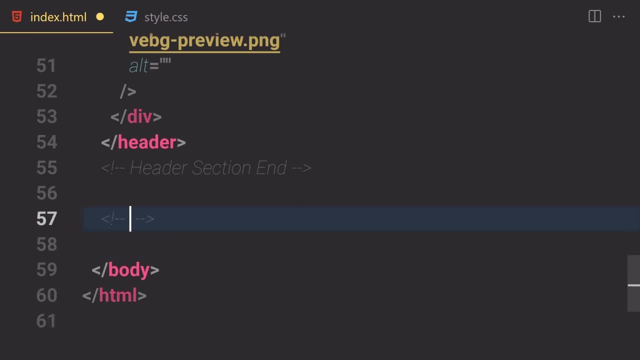 section and hey, so now let's just get into into into html. and here i'm going to write a html, and here i'm going to write a html, and here i'm going to write a comment for myself, like comment for myself, like comment for myself, like, uh, what popularity section start? 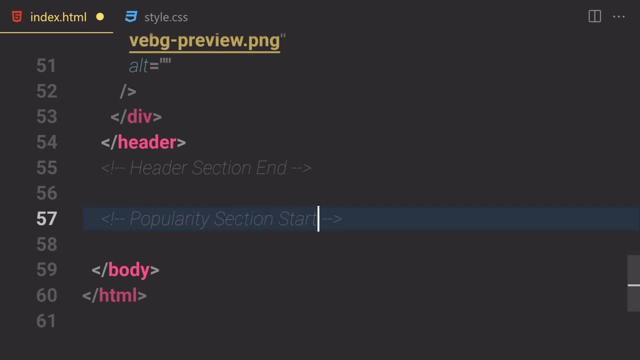 uh, what popularity section start. uh, what popularity section start. popularity section start would be fine. popularity section start would be fine. popularity section start would be fine, and i'm going to duplicate that and i'm, and, i'm going to duplicate that and i'm, and, i'm going to duplicate that and i'm going to set that to like n. going to set that to like n, going to set that to like n, and inside there we are going to be, and inside there we are going to be, and inside there we are going to be creating a section with the class of, creating a section with the class of. 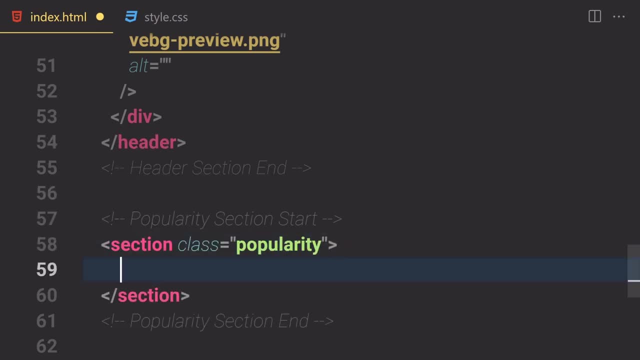 creating a section with the class of popularity: popularity, popularity inside this popularity section. we are inside this popularity section. we are inside this popularity section. we are going to be creating a new container, going to be creating a new container, going to be creating a new container with the class of popularity one. 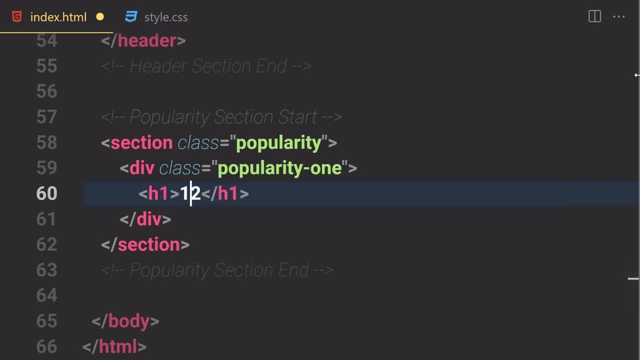 with the class of popularity, one with the class of popularity, one inside this popularity one. i'm going to inside this popularity one. i'm going to inside this popularity one. i'm going to write h1 with the write h1 with the write h1, with the text of 12k plus would be fine. and now, 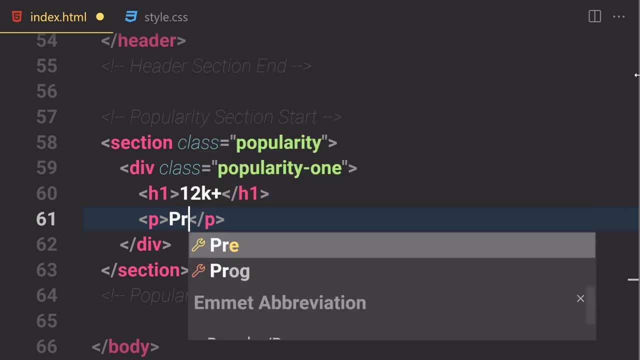 text of 12k plus would be fine. and now text of 12k plus would be fine. and now let's just create a paragraph with the. let's just create a paragraph with the. let's just create a paragraph with the class, or not a class, but a text of a. 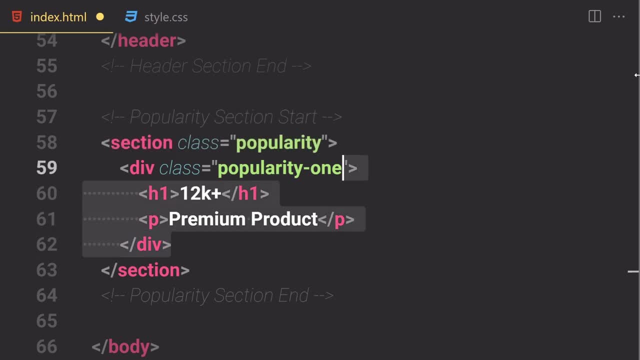 class or not a class, but a text of a class, or not a class, but a text of a premium product: premium product, premium product. okay, so i'm going to just duplicate this. okay, so i'm going to just duplicate this. okay, so i'm going to just duplicate this one two times. so this is going to be. 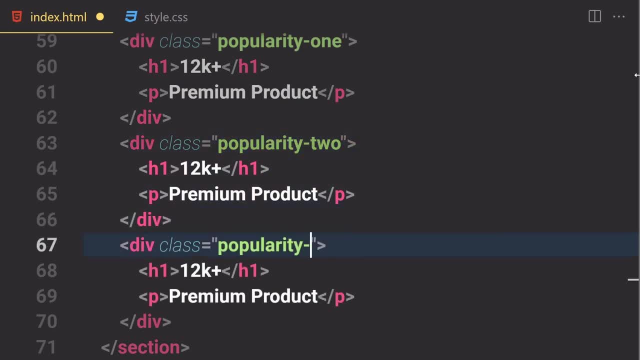 one two times. so this is going to be one two times. so this is going to be the popularity two and this is going to the popularity two and this is going to the popularity two and this is going to be the popularity three. okay, so, let's be the popularity three. okay, so let's. 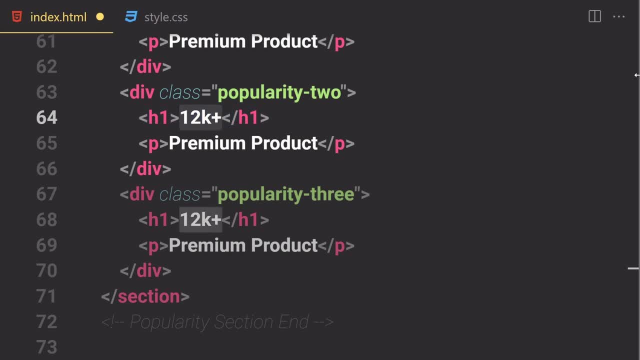 be the popularity three. okay, so let's just change this text to be like: just change this text to be like, just change this text to be like something else, something else, something else, uh, i don't know, 21 uh, 21k. uh, i don't know, 21 uh, 21k. 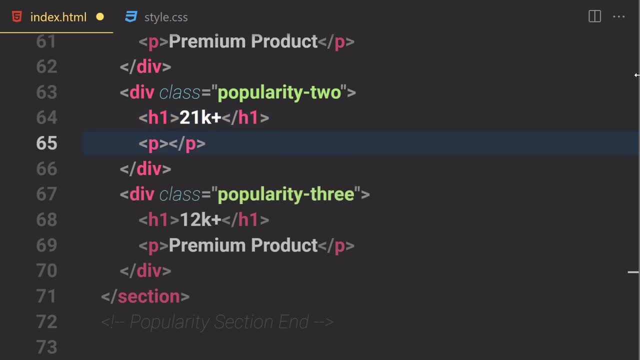 uh, i don't know, 21, uh, 21k or k would be fine, k plus, and also or k would be fine, k plus, and also or k would be fine, k plus. and also happy customers, customers, customers, customers, all right, so also change this text to. 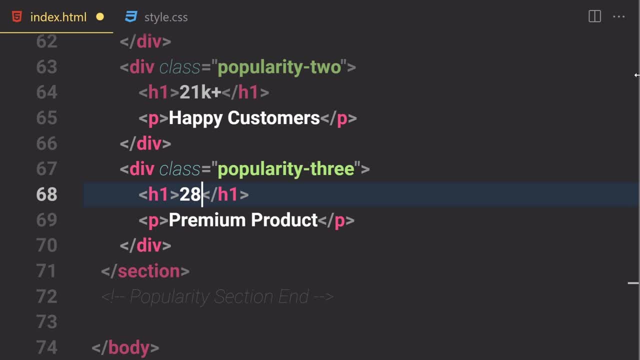 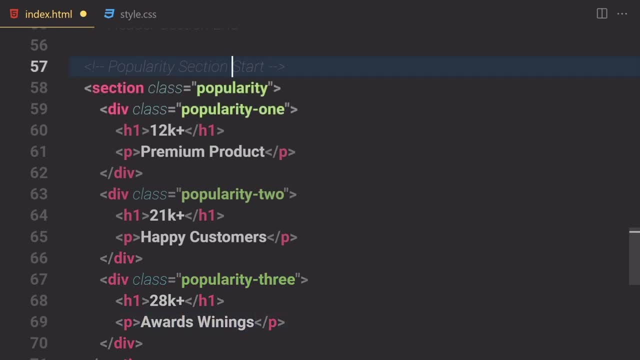 okay, so this is going to be it for okay, so this is going to be it for popularity section. so we have uh one popularity section. so we have uh one popularity section. so we have uh one div with a class of popularity inside. div with a class of popularity inside. 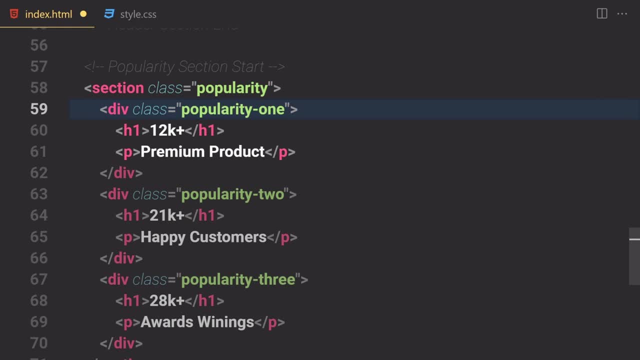 div with a class of popularity. inside there we have three more divs. so with there, we have three more divs. so with there we have three more divs. so with the class of popularity one, two and the class of popularity one, two and the class of popularity one, two and three, and then we have a little bit of 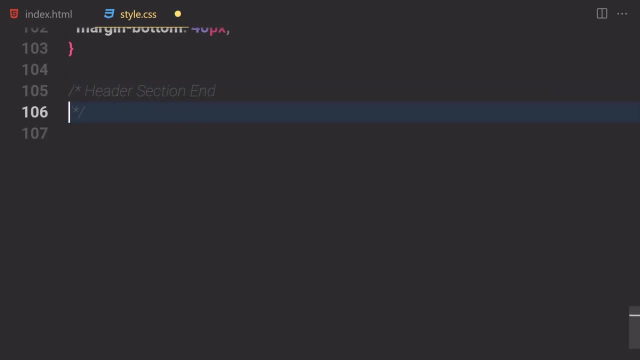 three, and then we have a little bit of three and then we have a little bit of text inside this. now, let's just try a text inside this now. let's just try a text inside this. now, let's just try a little bit and let's just write, or: 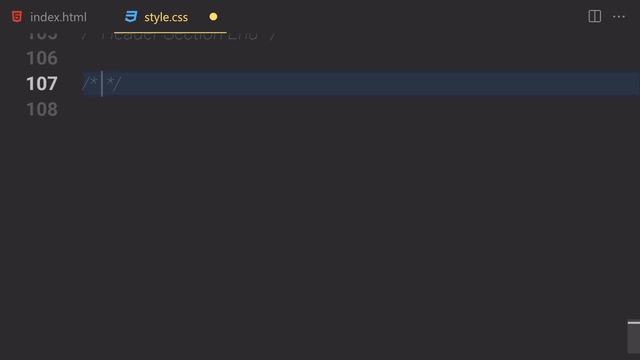 little bit and let's just write. or little bit and let's just write, or comment first of all. comment, first of all comment. first of all, i'm going to write a comment for myself. i'm going to write a comment for myself. i'm going to write a comment for myself like, uh, popularity. 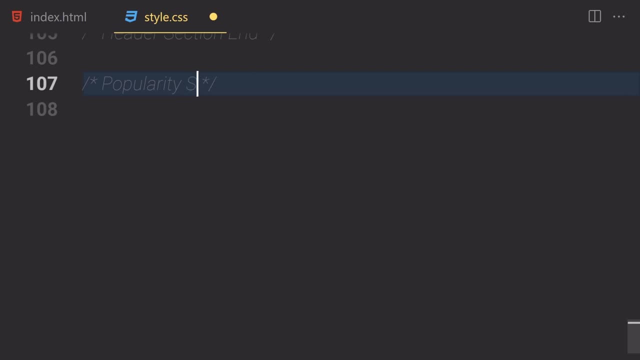 like uh popularity. like uh popularity: eo p? u l a r i t, eo p u l a r i t eo p u l a r i t. popularity section start and i'm going to popularity section start and i'm going to popularity section start and i'm going to duplicate that and i'm going to change it. 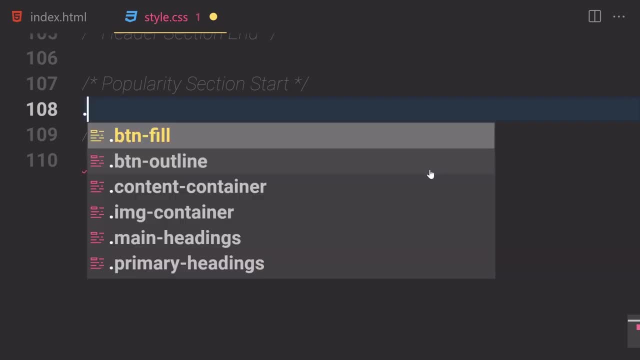 duplicate that and i'm going to change it. duplicate that and i'm going to change it to popularity section end and first of to popularity section end and first of to popularity section end and first of all, let's just start working on our all. let's just start working on our. 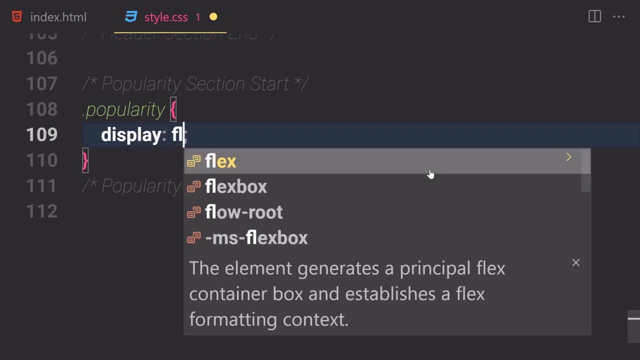 all, let's just start working on our popularity section, popularity section, popularity section- and let's just put our display of flex on. and let's just put our display of flex on, and let's just put our display of flex on it. justify content will be now set to. 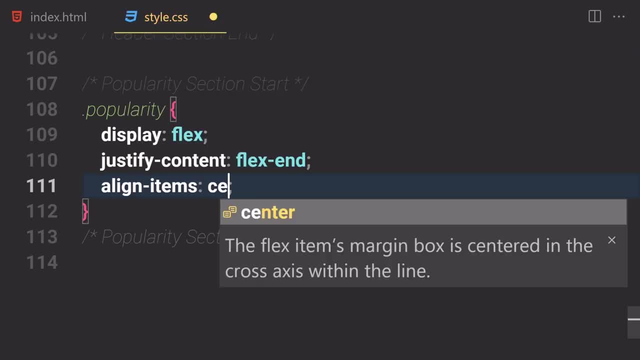 it. justify content will be now set to it. justify content will be now set to flex. and because we want to push there flex, and because we want to push there flex, and because we want to push there to the end and align items will be now to the end and align items will be now. 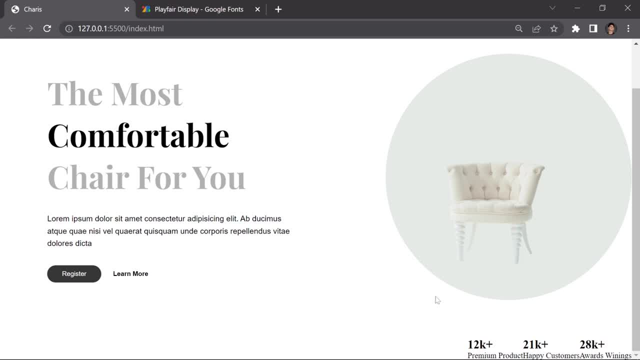 to the end and align. items will be now set to center. so if you sell that set to center, so if you sell that set to center, so if you sell that, and we cannot see that, and we cannot see that, and we cannot see that, why not? let's just see. why can't all? 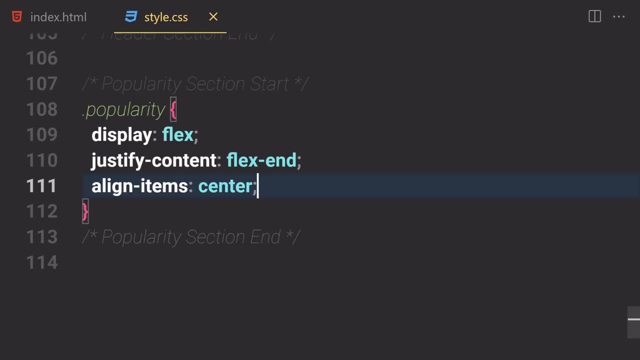 why not? let's just see why can't all? why not? let's just see why can't all? right, so we can see that right here. right, so we can see that right here. right, so we can see that right here, uh, underneath. so what do we have to do? 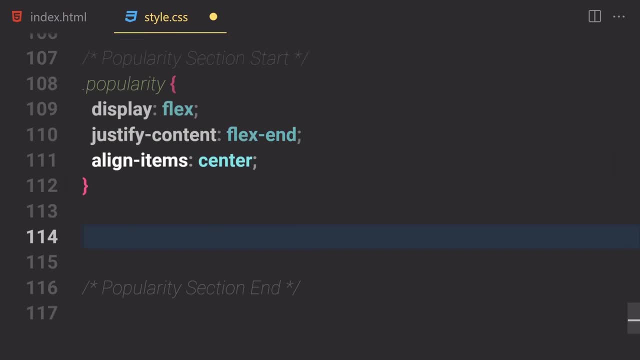 uh, underneath. so what do we have to do? uh, underneath. so what do we have to do? let's just select our div inside that. let's just select our div inside that. let's just select our div inside that popularity section, which is popularity section, which is popularity section, which is, uh, these div like uh, popularity one, two. 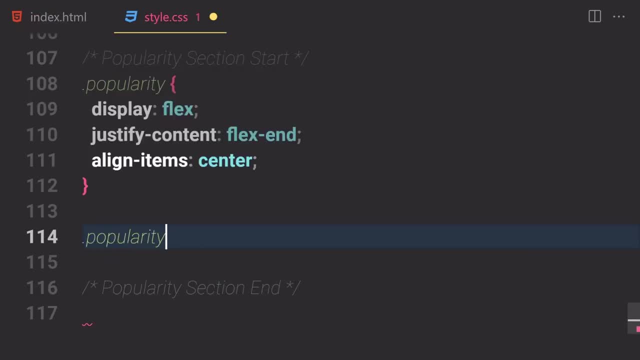 uh, these div like uh popularity one, two. uh, these div like uh popularity one, two and three divs. so let's just select that and three divs. so let's just select that and three divs. so let's just select that. i'm gonna write a popularity and let's i'm gonna write a popularity and let's- i'm gonna write a popularity and let's just select all of the divs, which is just select all of the divs. which is just select all of the divs. which is inside there, i'm gonna write a margin. 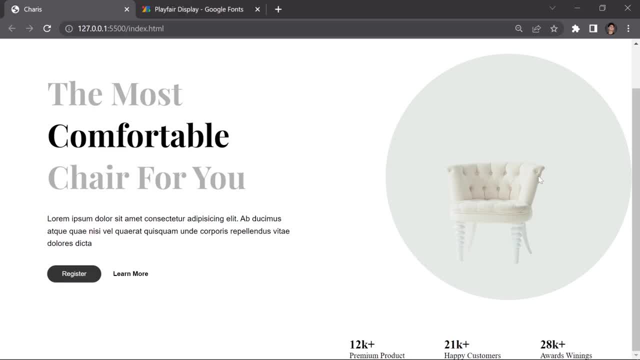 inside there. i'm gonna write a margin inside there. i'm gonna write a margin right for them. like five remote we find, right for them. like five remote, we find right for them. like five remote, we find. and now, if you save that and this is how, and now, if you save that and this is how. 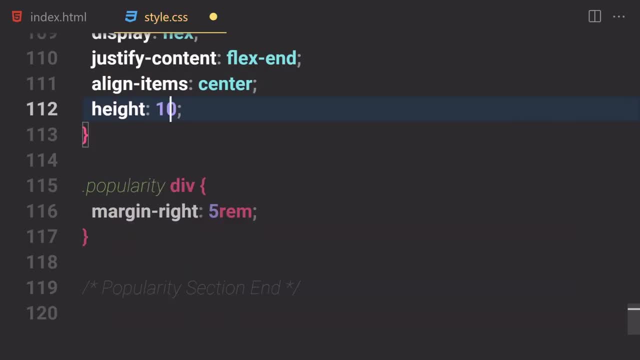 and now, if you save that, and this is how it looks like, it looks like, it looks like, and, oh, you know what, first of all let. and oh, you know what first of all let, and oh, you know what. first of all, let me just give him a height of like 100. 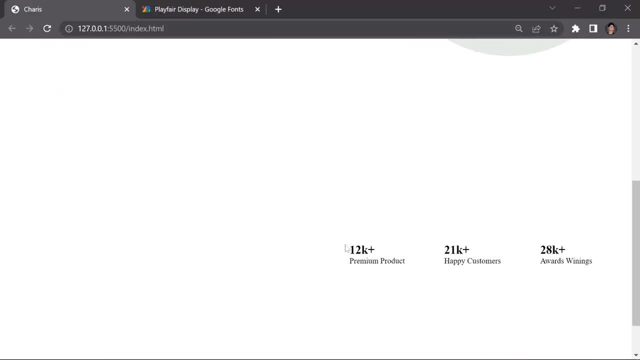 me just give him a height of like 100 me, just give him a height of like 100 vh, so you guys can see everything a bit vh. so you guys can see everything a bit vh. so you guys can see everything a bit clear, clear, clear. now it's here, but it will just take its 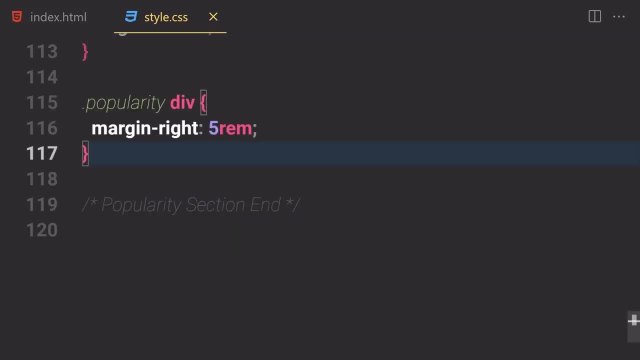 now it's here, but it will just take its. now it's here, but it will just take its place once we remove that uh 100 pixel place, once we remove that uh 100 pixel place, once we remove that uh 100 pixel of viewport height. so i just want to. 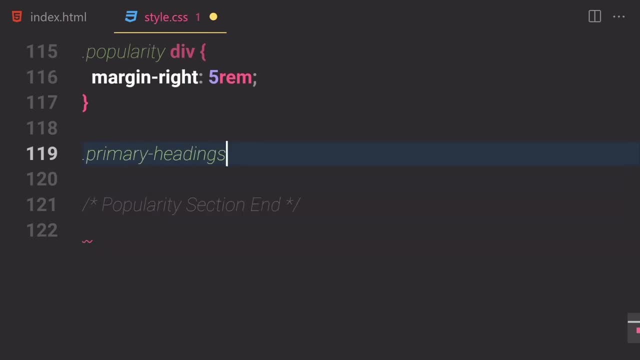 of viewport height, so i just want to of viewport height. so i just want to show everything in a one viewport. so show everything in a one viewport. so show everything in a one viewport. so let's just select our popularity, not. let's just select our popularity, not. 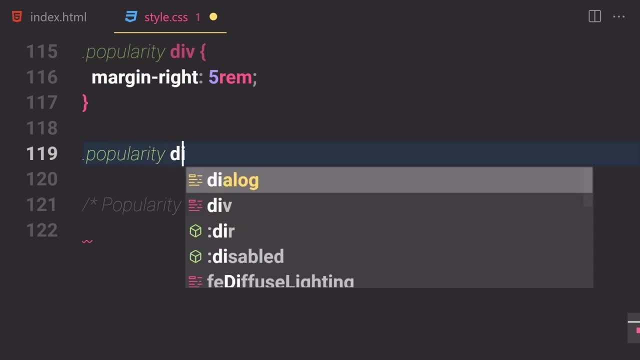 let's just select our popularity: not primary headings but um primary headings, but um primary headings but um popularity. and inside there we are going popularity, and inside there we are going popularity. and inside there we are going to be selecting each of their h1, to be selecting each of their h1. to be selecting each of their h1. so we are going to be just increasing the. so we are going to be just increasing the. so we are going to be just increasing the font size to be like i don't know three. font size: to be like i don't know three. 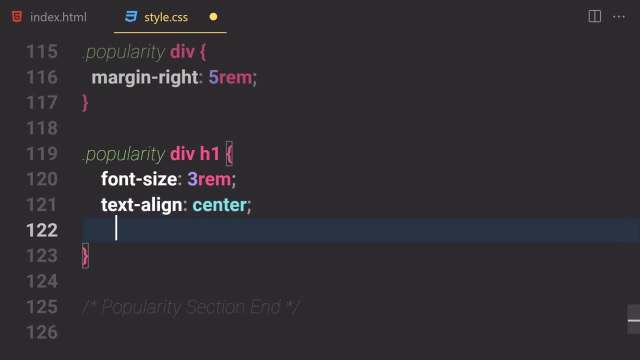 font size to be like i don't know three. ram and text alignment will be now set. ram and text alignment will be now set. ram and text alignment will be now set to totally center and i'm going to also to totally center and i'm going to also. 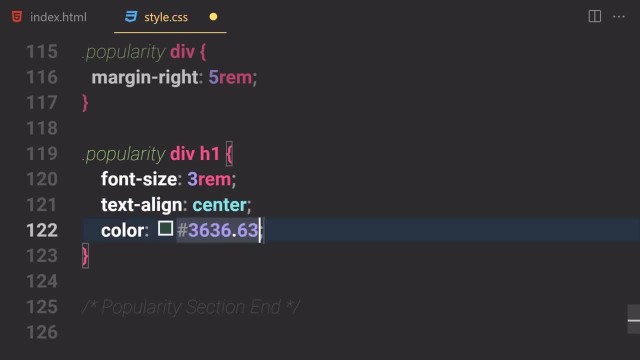 to totally center and i'm going to also change the color to be three six, three. change the color to be three six three. change the color to be three six, three, six and three, six, six and three, six, six and three, six. uh, let's just remove that period from. 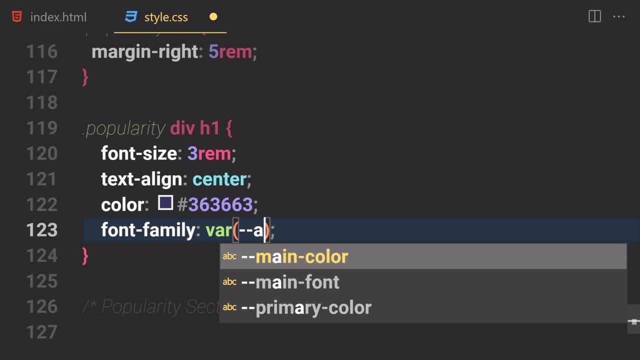 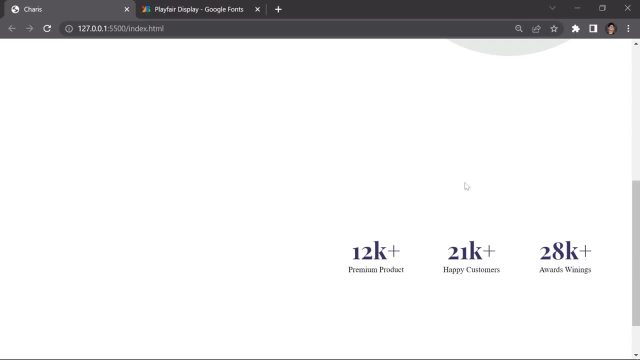 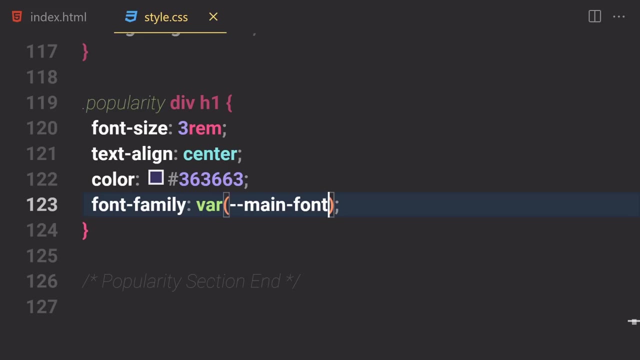 uh, let's just remove that period from. uh, let's just remove that period from there, there, there, and for family, i'm going to change that and for family, i'm going to change that and for family, i'm going to change that. i do, i do, i do, you know, i'm going to just stick to that. 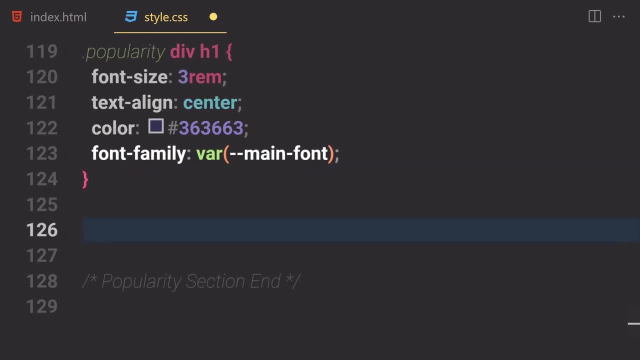 you know i'm going to just stick to that. you know i'm going to just stick to that. if you want to choose your own kind of a, if you want to choose your own kind of a, if you want to choose your own kind of a color, so you can also provide that now. 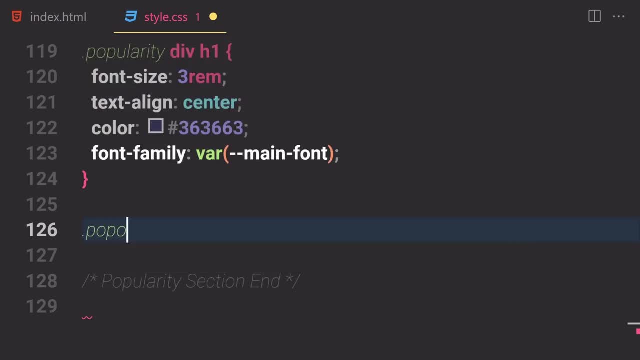 color, so you can also provide that now. color, so you can also provide that. now. let's just select all of their, let's just select all of their, let's just select all of their paragraph, which is inside their paragraph, which is inside their paragraph, which is inside their popularity. p o p u l a r t y. popularity p o p u l a r t y. popularity p o p? u l a r t y div, and all of their popularity div and all of their popularity div and all of their popularity paragraphs. so now, let's just select that paragraphs. so now, let's just select that. 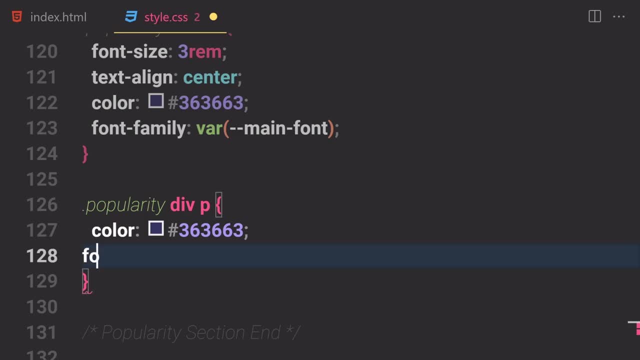 paragraphs. so now let's just select that. i'm going to copy this color from there. i'm going to copy this color from there. i'm going to copy this color from there. i'm going to paste it right here and i'm. i'm going to paste it right here and i'm. i'm going to paste it right here and i'm going to also change the font family to going to also change the font family, to going to also change the font family to be censored. so if you sell that, be censored. so if you sell that. be censored. so if you sell that, and this is how it looks like for now, and this is how it looks like for now, and this is how it looks like for now, okay, so now i'm going to just remove. okay, so now i'm going to just remove. 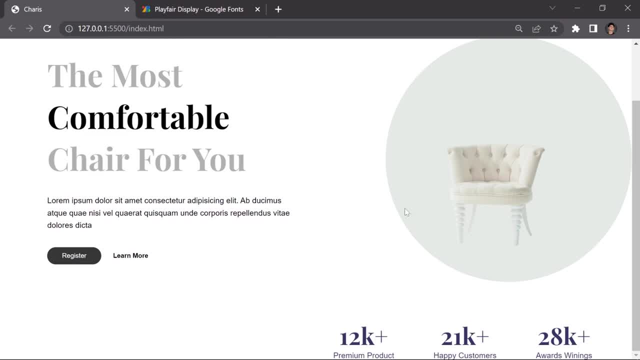 okay, so now i'm going to just remove that hide from there. so let's just that hide from there. so let's just that hide from there. so let's just remove that hide, save it. remove that hide, save it, remove that hide, save it. and this is how it looks, like you know. 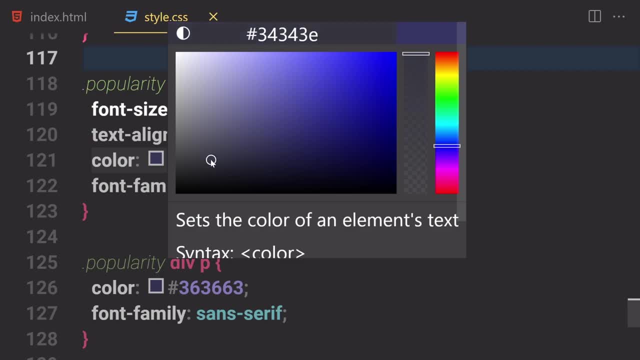 and this is how it looks like you know. and this is how it looks like you know. i'm going to turn this color to. i'm going to turn this color to. i'm going to turn this color to something else. it's looking awful, something else. it's looking awful. 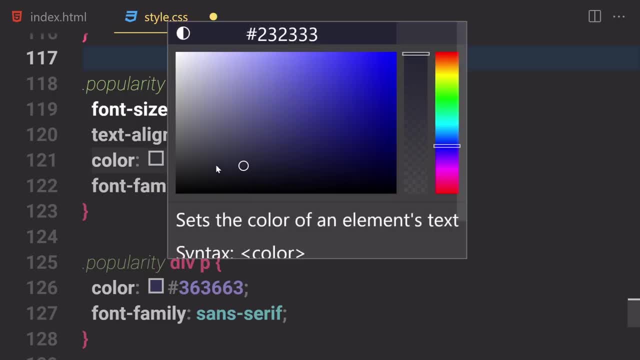 something else, it's looking awful. so if you sell that, yeah, this color is so. if you sell that, yeah, this color is so. if you sell that, yeah, this color is fine, fine, fine, ah, not that one. ah, not that one. ah, not that one. let's just copy this color. 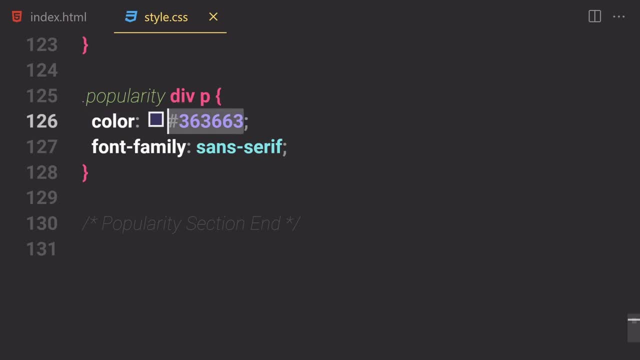 let's just copy this color. let's just copy this color. i'm going to paste it in here as well. i'm going to paste it in here as well. i'm going to paste it in here as well. uh, like so. so i'm going to paste it. uh like so, so i'm going to paste it. uh like so, so i'm going to paste it. yeah, it's looking better anyway. so we, yeah, it's looking better anyway. so we, yeah, it's looking better anyway. so we are totally done with this popularity, are totally done with this popularity. 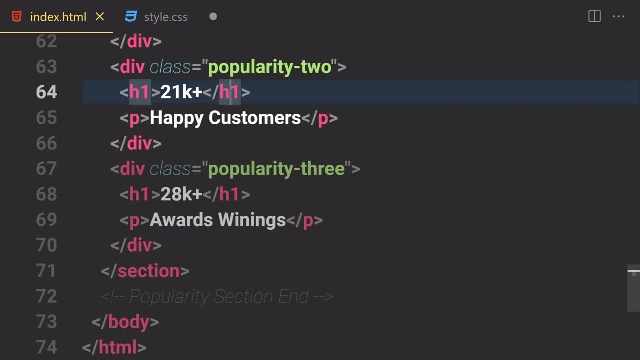 are totally done with this popularity section as well. so what else do you have? section as well. so what else do you have? section as well. so what else do you have to do now? let's just start working on to do now. let's just start working on. 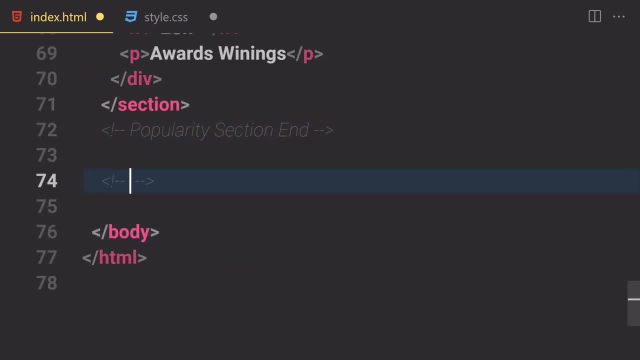 to do now. let's just start working on our products container sections. so, let's our products container sections. so let's our products container sections. so let's just write a comment for yourself, like, just write a comment for yourself. like, just write a comment for yourself, like: products, um, what product section start? 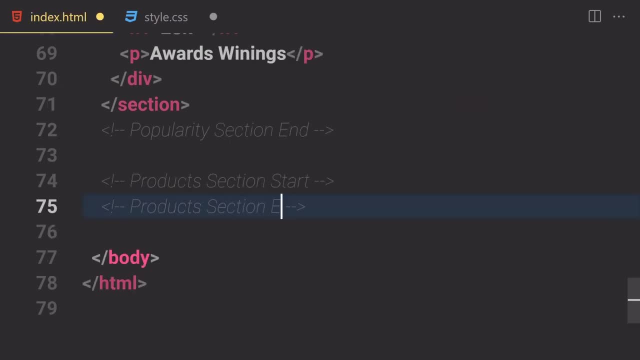 products um what product section start. products um what product section start, start and duplicate that. and product uh start and duplicate that. and product uh start and duplicate that. and product uh section end. okay. so inside there we are section end. okay. so inside there we are section end. okay, so inside there we are going to be writing a lot of html, so we going to be writing a lot of html. so we going to be writing a lot of html, so we are going to be writing a section first. are going to be writing a section first. are going to be writing a section first of all with the class of products. 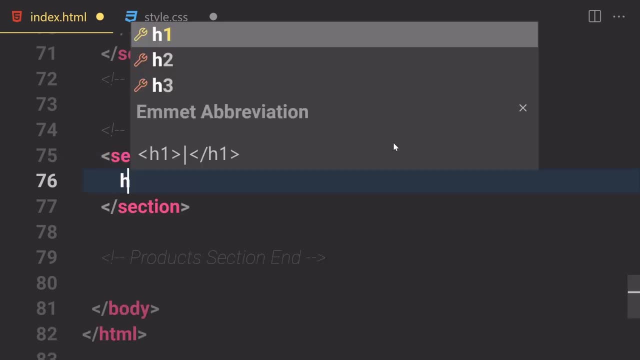 of all with the class of products, of all with the class of products, products, and then container inside this products and then container inside this products and then container inside this products container- we are going to be products- and then container inside this products container. we are going to be writing h1 with the. 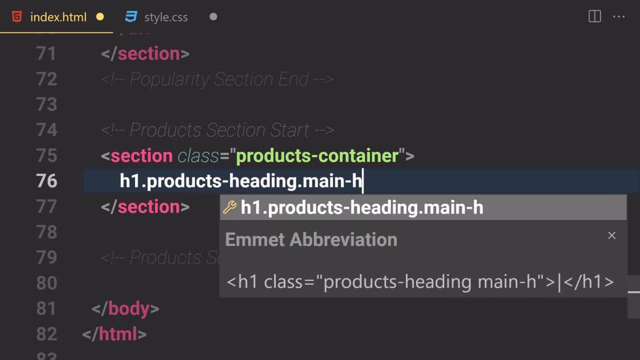 writing h1 with the writing h1 with the class of products heading and also the class of products heading and also the class of products heading and also the main headings. okay, so inside there i'm main headings. okay. so inside there i'm main headings. okay, so inside there i'm going to zoom out of it. 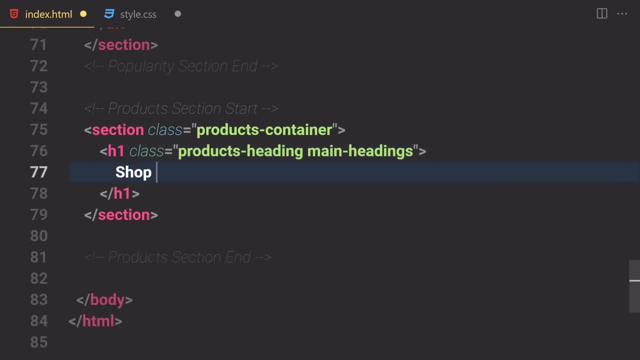 going to zoom out of it. going to zoom out of it inside the h1. we are going to be writing inside the h1. we are going to be writing inside the h1. we are going to be writing it not h1, but shop, a popular popu lar. 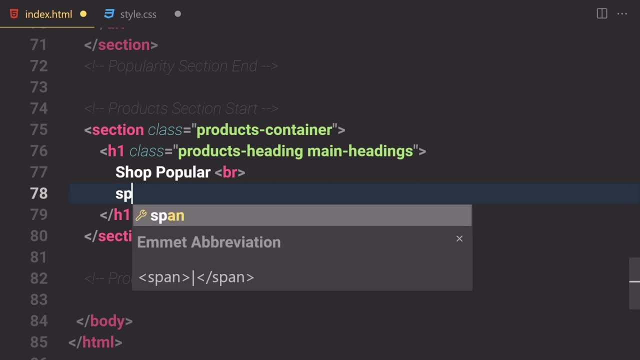 it not h1, but shop a popular popu lar. it not h1, but shop a popular popu lar, like so. and i'm going to put a br tag in like so, and i'm going to put a br tag in like so, and i'm going to put a br tag in there. and now let me just put a span in. 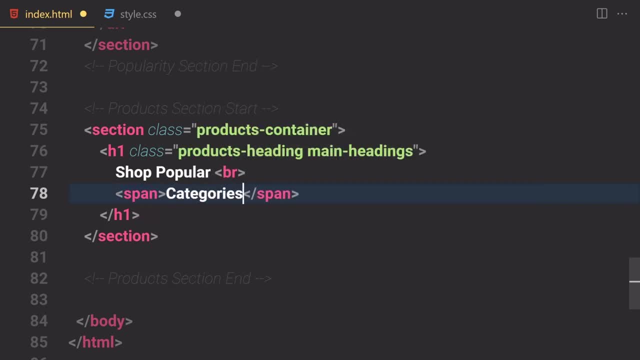 there, and now let me just put a span in there. and now let me just put a span in here, and categories here and categories here and categories like so underneath this h1. what do we like so underneath this h1? what do we like so underneath this h1? what do we have to do? we are going to be writing. 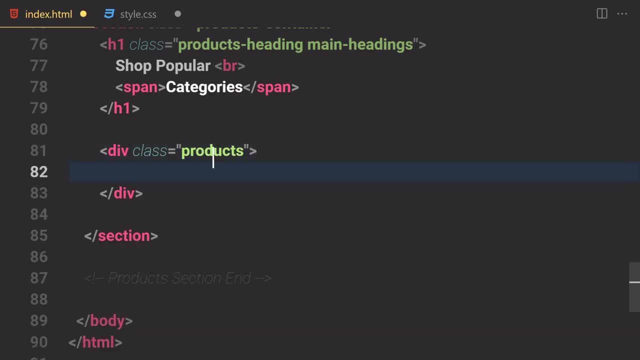 have to do, we are going to be writing, have to do, we are going to be writing: each of the products containers, so each of the products containers, so each of the products containers, so products inside there we are going to be. products inside there we are going to be. 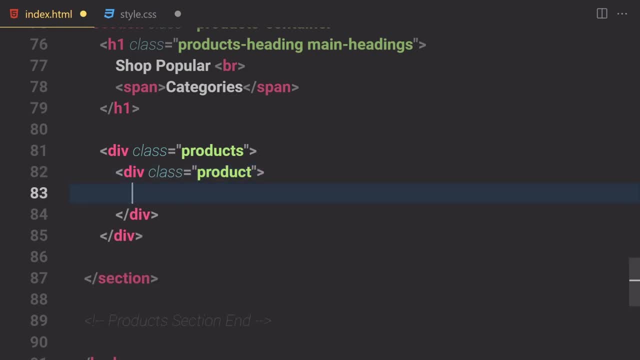 products. inside there, we are going to be using just a regular, using just a regular, using just a regular product singular product to be precise. product singular product to be precise. product singular product to be precise. inside there, we are going to be using a product singular product to be precise. inside there, we are going to be using a. 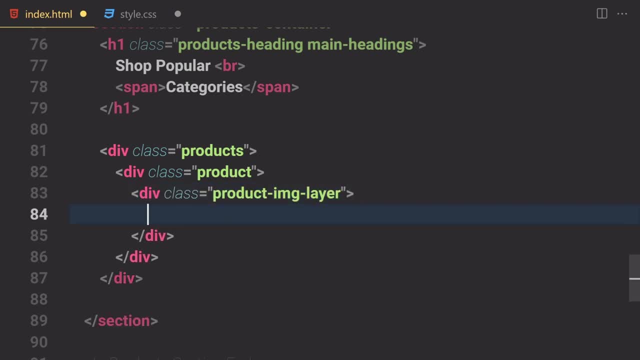 product, singular product, to be precise. inside there we are going to be using a product image, product image, product image, a layer. okay, so this is going to be the a layer. okay, so this is going to be the a layer. okay, so this is going to be the layer for image. inside there we are going. 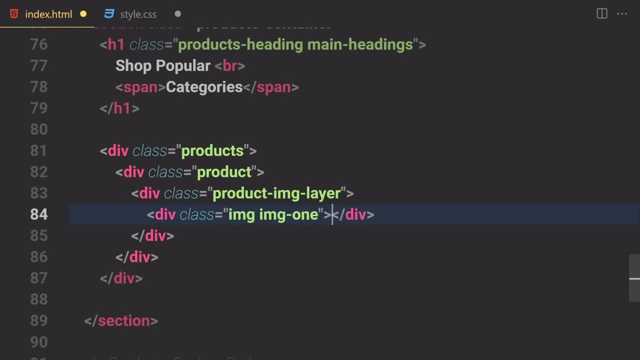 layer for image inside there we are going. layer for image inside there we are going to be using an image and then img1. so to be using an image, and then img1, so to be using an image, and then img1. so this is going to be the first image. 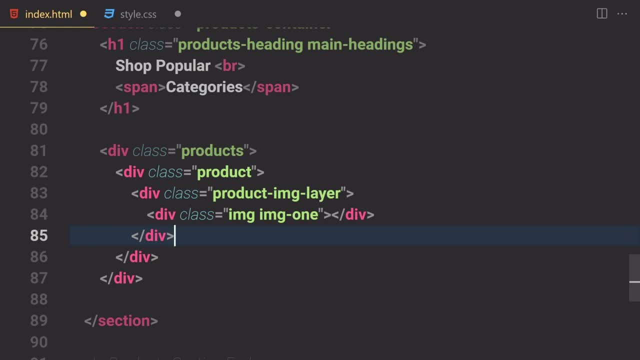 this is going to be the first image. this is going to be the first image anyways, so what do we have to do in this anyways? so what do we have to do in this anyways? so what do we have to do in this case? we want to duplicate that. 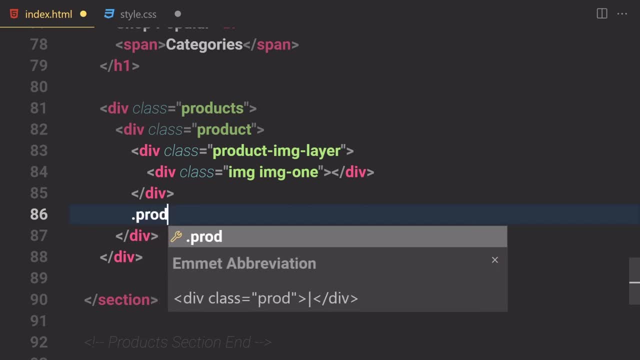 case, we want to duplicate that case. we want to duplicate that. so. so, underneath this div, we are going so. so, underneath this div, we are going so. so, underneath this div, we are going to be creating a new div with a class of. to be creating a new div with a class of. 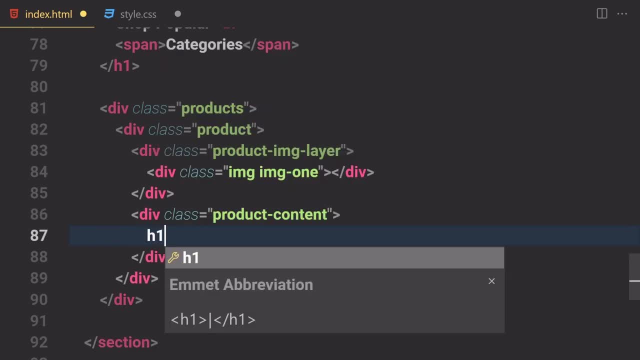 to be creating a new div with a class of product content. so, inside this product product content. so inside this product product content. so, inside this product content, we are going to be writing h1 content. we are going to be writing h1 content. we are going to be writing h1 with a class of product name. so i'm 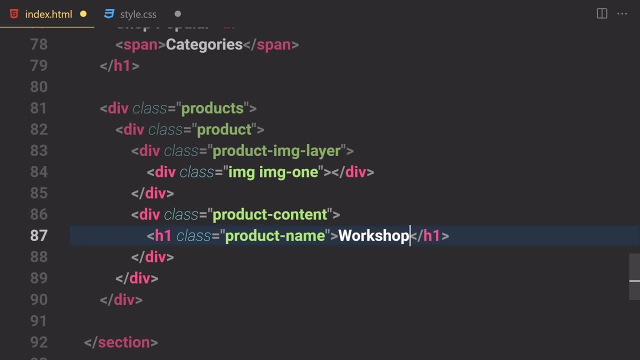 with a class of product name. so i'm with a class of product name, so i'm going to just write like workshop. going to just write like workshop, going to just write like workshop: chair, chair, chair. okay, so, workshop chair and i'm going to. okay, so, workshop chair and i'm going to. 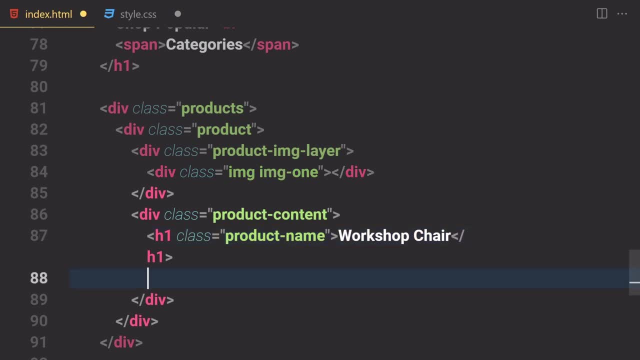 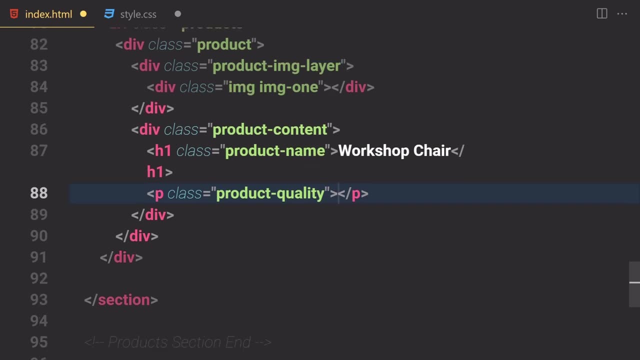 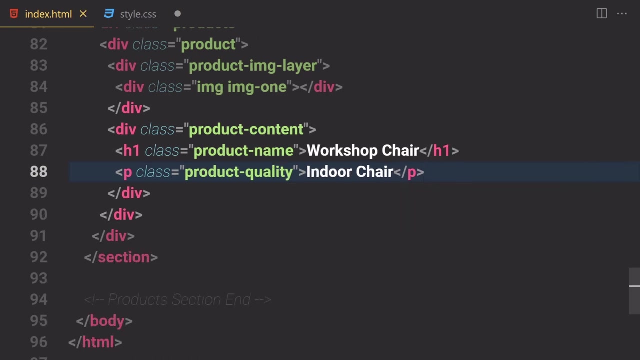 okay, so workshop chair and i'm going to duplicate this line of code. or you know, duplicate this line of code. or you know, duplicate this line of code. or you know, and in door chair and in door chair and in door chair chair, like so so if you sell that, chair like so, so if you sell that chair like so, so if you sell that, and this is how it looks like. so now i'm, and this is how it looks like. so now i'm, and this is how it looks like. so now i'm going to just duplicate this product. 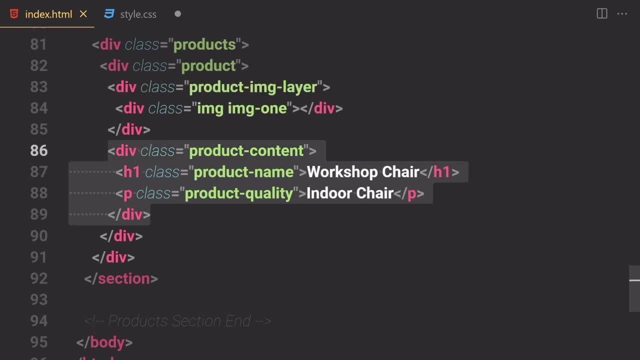 going to just duplicate this product. going to just duplicate this product. content two times so. content two times so. content two times so this is going to be the first time. or you, this is going to be the first time, or you this is going to be the first time, or you know what? 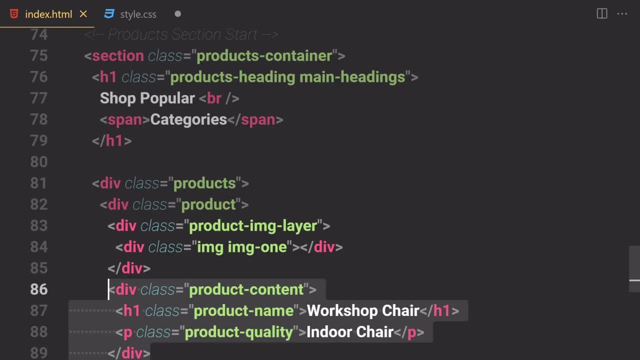 know what? know what we're not going to be duplicating there. we're not going to be duplicating there. we're not going to be duplicating there. so, so, so, you know what i'm going to duplicate this. you know what i'm going to duplicate this. 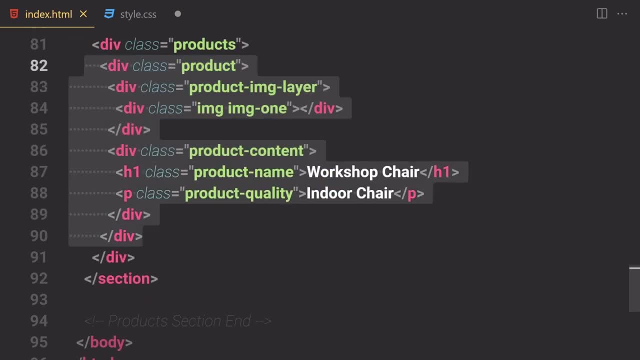 you know what? i'm going to duplicate this product from here, product from here, product from here to here. so this is going to be the first to here. so this is going to be the first to here. so this is going to be the first product. then we have a second one, and 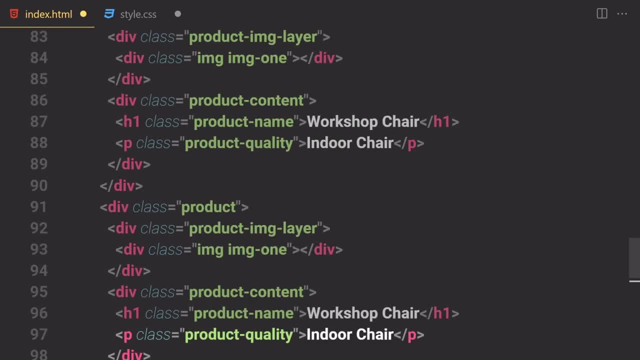 product, then we have a second one, and product, then we have a second one and the third one. okay, so the third one, okay, so the third one, okay. so this is going to be the first one and we, this is going to be the first one and we. 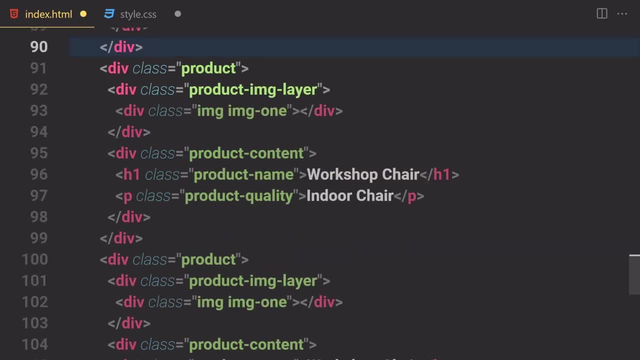 this is going to be the first one, and we are totally done with that right here. so are totally done with that right here. so are totally done with that right here. so this is going to be the second one, and this is going to be the second one, and 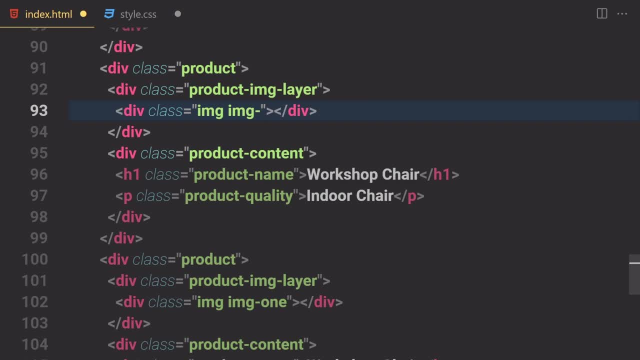 this is going to be the second one, and then we have to change this one, from then we have to change this one, from then we have to change this one from image one to image one, to image one, to image two. okay, so we also, you know what, 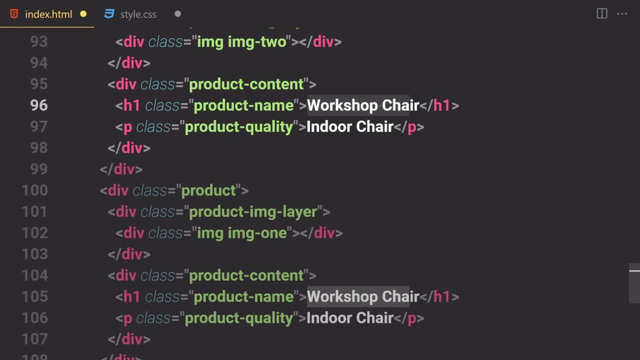 image two. okay, so we also you know what. image two. okay, so we also you know what this is going to be the same like this is going to be the same like this is going to be the same like workshop chair and indoor chair. workshop chair and indoor chair. 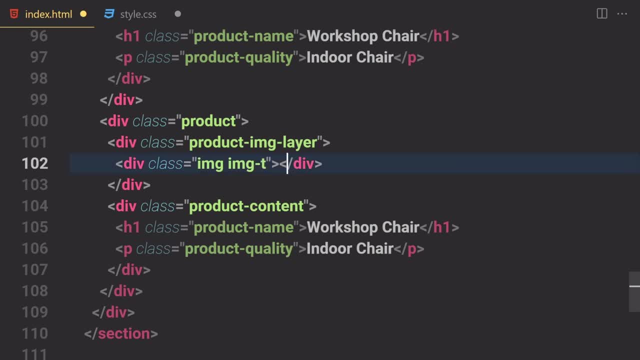 workshop chair and indoor chair. let's just also change this image, uh one. let's just also change this image, uh one. let's just also change this image- uh one- to be image three in this case. okay, to be image three in this case. okay, to be image three in this case. okay, everything is now fine. so underneath. 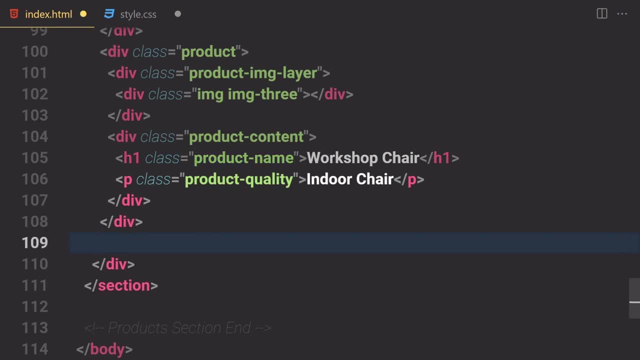 everything is now fine. so underneath: everything is now fine. so underneath this div. what i'm going to do is that this div. what i'm going to do is that this div. what i'm going to do is that i'm going to just create a section, or. 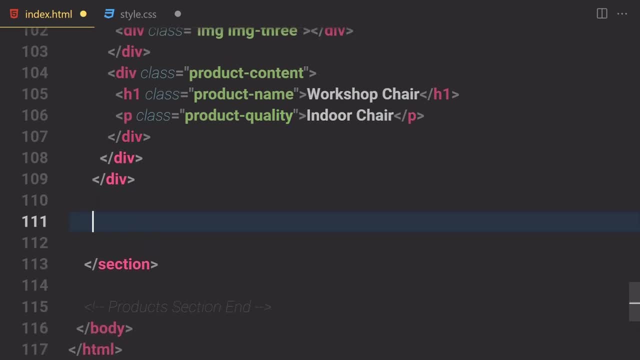 i'm going to just create a section. or i'm going to just create a section. or you know what outside from that div, but you know what outside from that div, but you know what outside from that div, but inside that, inside that, inside that, uh section. so we are going to be. 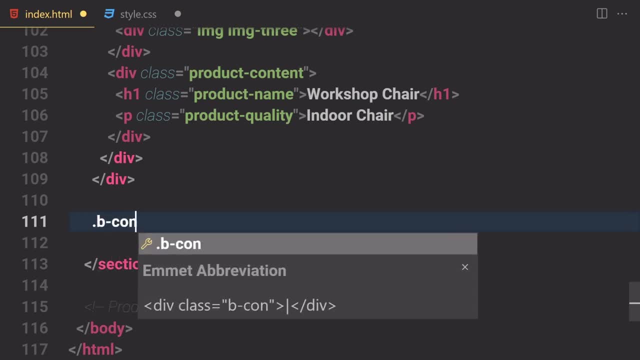 uh section. so we are going to be uh section. so we are going to be creating a new section or div. creating a new section or div, creating a new section or div with the class of b and then container with the class of b, and then container with the class of b and then container for buttons, containers. so we are going. 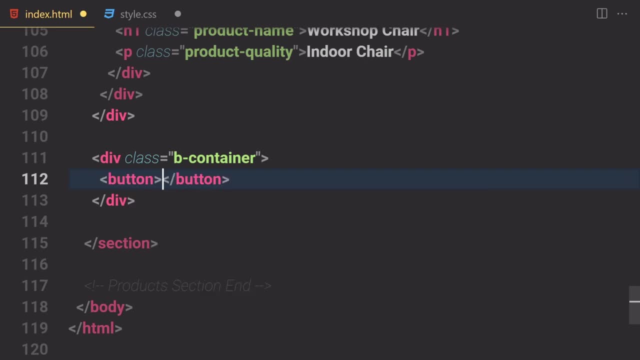 for buttons containers. so we are going for buttons containers. so we are going to be just placing our button, to be just placing our button, to be just placing our button here. we are going to be placing our here. we are going to be placing our here. we are going to be placing our html entity. so, first of all, i'm going to 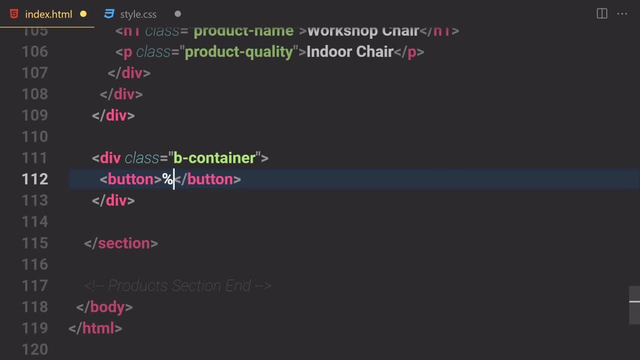 html entity. so, first of all, i'm going to html entity. so first of all, i'm going to just write an ensemble, and some, oh my, just write an ensemble. and some, oh my, just write an ensemble. and some, oh, my goodness. so we are going to be writing. 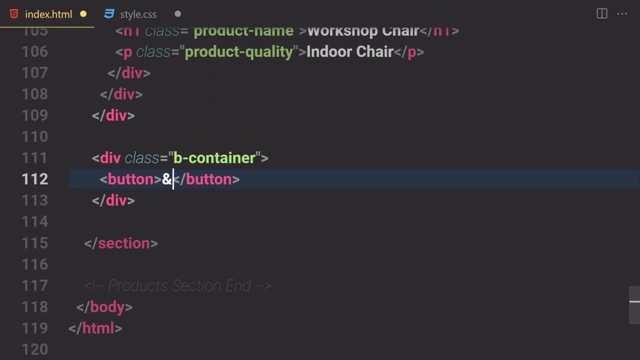 goodness, so we are going to be writing. goodness, so we are going to be writing an answer. where is my end symbol? an answer, where is my end symbol? an answer, where is my end symbol? yeah, there we go, so we are going to be. yeah, there we go, so we are going to be. 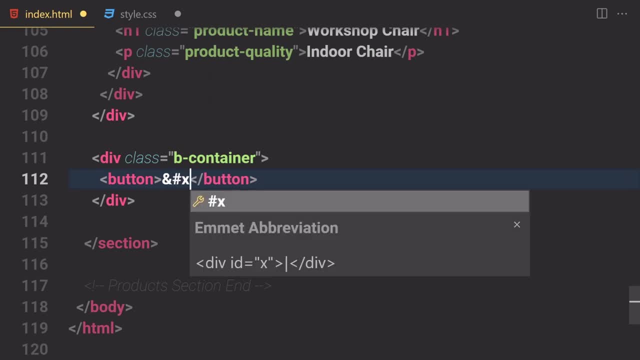 yeah, there we go. so we are going to be writing an end symbol and then the pound writing an end symbol, and then the pound writing an end symbol, and then the pound symbol. then x 2, 1, 9, 0. okay, so this is symbol. then x 2, 1, 9, 0. okay, so this is. 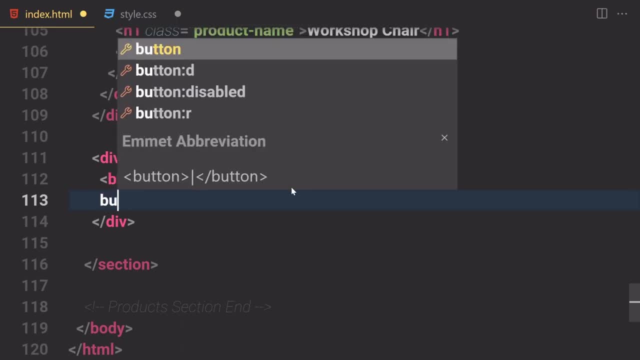 symbol. then: x, 2, 1, 9, 0. okay, so this is going to be the first arrow, and now going to be the first arrow, and now going to be the first arrow, and now let's just write a new button, so i'm: let's just write a new button, so i'm. 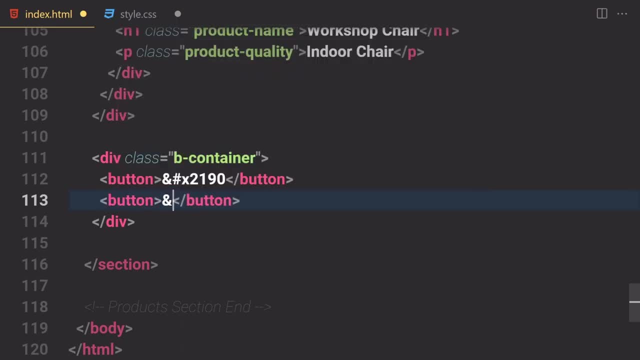 let's just write a new button. so i'm gonna write a button and let's just gonna write a button, and let's just gonna write a button and let's just provide our end symbol, and then r a provide our end symbol, and then r a provide our end symbol, and then r a double r, and then just close it, okay, so 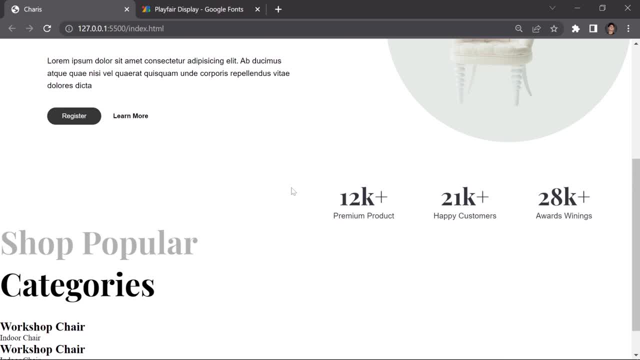 double r and then just close it. okay. so double r and then just close it. okay, so i'm gonna also, i'm gonna also, i'm gonna also close the other one right here. so if close the other one right here, so if close the other one right here, so if it's our file and it will not use that, 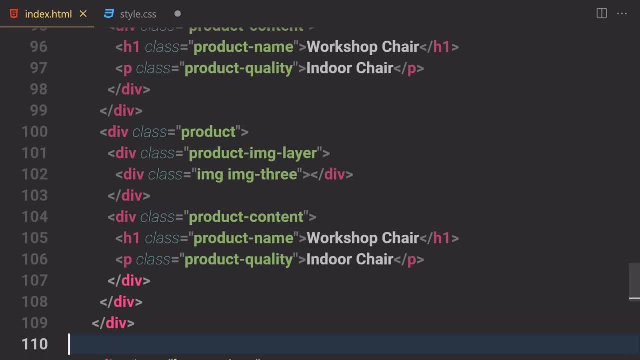 it's our file and it will not use that. it's our file and it will not use that. arrow which you cannot see right away. arrow which you cannot see right away. arrow which you cannot see right away, but this is going to be it for, or html. but this is going to be it for or html. but this is going to be it for or html. so now, let's just style that a bit. so so now, let's just style that a bit. so so now, let's just style that a bit. so, first off, you know what? let me just 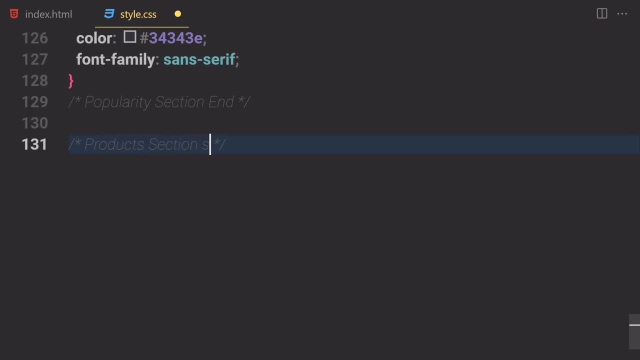 first off, you know what? let me just first off you know what? let me just write a comment for myself, like products. write a comment for myself like products. write a comment for myself, like products. section, section, section, start. okay, so this is going to be the start. okay, so this is going to be the. 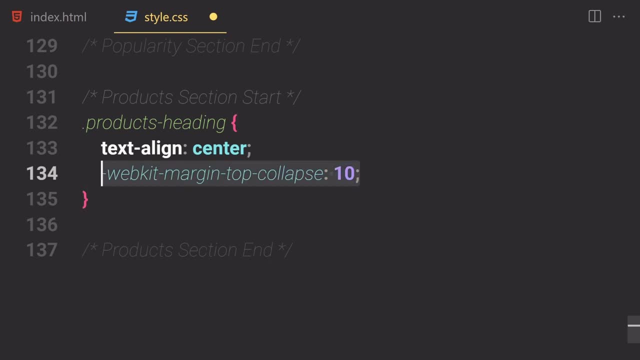 start. okay, so this is going to be the center and margin for the top. i'm going center and margin for the top. i'm going center and margin for the top. i'm going to give him like to give him like to give him like: uh, margin, top. i'm going to give him like 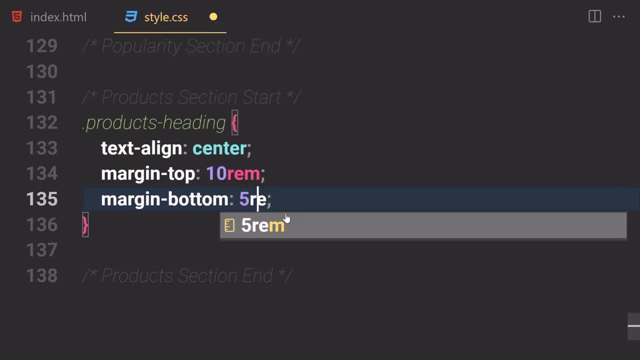 uh, margin top. i'm going to give him like uh, margin top. i'm going to give him like 10 ram and margin for the bottom. i'm 10 ram and margin for the bottom. i'm 10 ram and margin for the bottom. i'm going to give him like fire frame and. 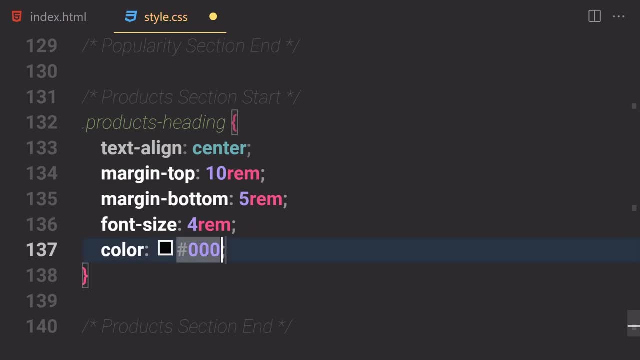 going to give him like fire frame and going to give him like fire frame and font size will be now set to 4 ram and font size will be now set to 4 ram and font size will be now set to 4 ram and color will be now, in this case, set to. 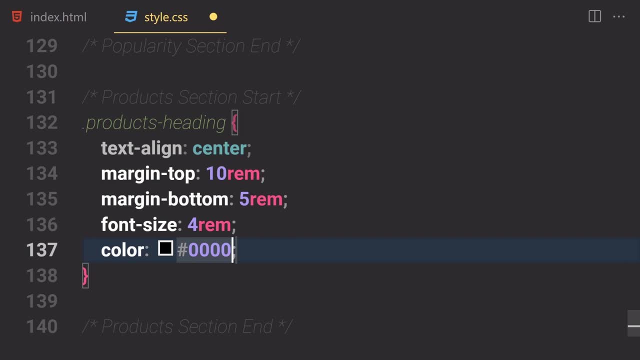 color will be now, in this case, set to. color will be now set to 4 ram and color will be now set to like uh three, like uh three, like uh three zeros, and then four, five, six and four zeros, and then four, five, six and four zeros, and then four, five, six and four f- kind of that bluish kind of color. so 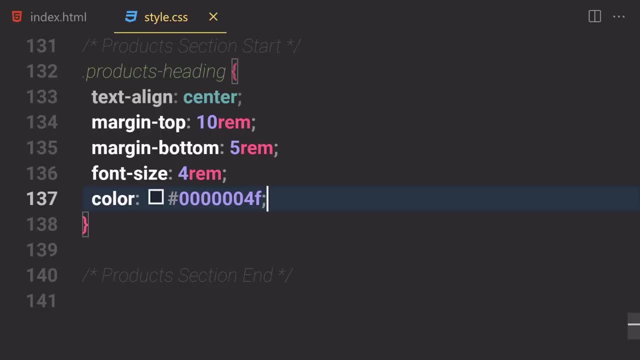 f kind of that bluish kind of color. so f kind of that bluish kind of color. so if you sell them, and this is how if you sell them, and this is how if you sell them, and this is how currently things looks like, all right, so 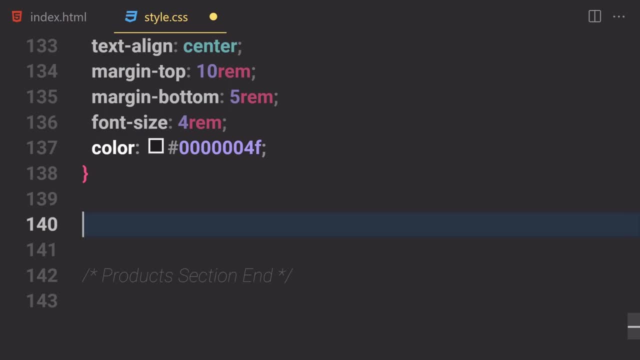 currently things looks like all right. so currently things looks like all right. so that was it for our products heading. that was it for our products heading. that was it for our products heading. let's just start working on our spain. so let's just start working on our spain. so. 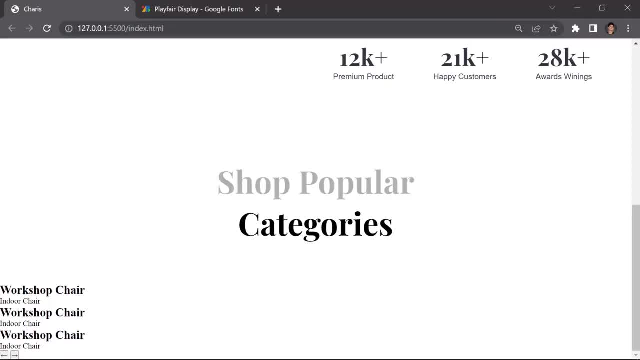 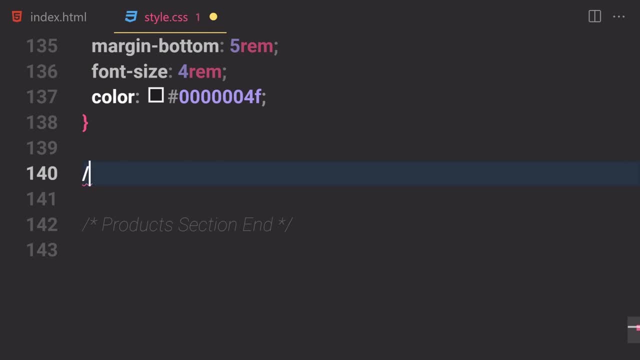 let's just start working on our spain. so we want to make that blank. i guess we want to make that blank. i guess we want to make that blank. i guess to totally center flex ramp will be now to totally center flex ramp will be now to totally center flex ramp will be now set to wrap and justify content will be. 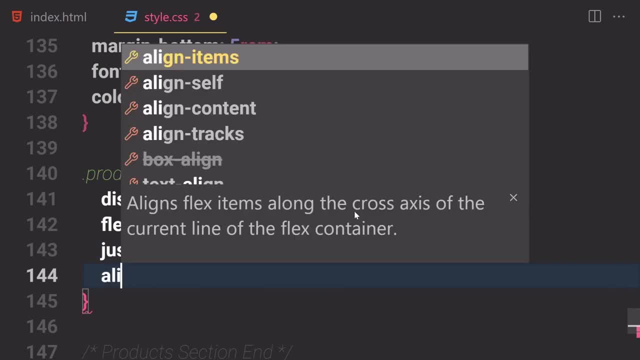 set to wrap and justify content will be set to wrap and justify content will be now. set to now. set to now. set to uh. space around uh. space around uh. space around and align items. i'm going to set that and align items. i'm going to set that. 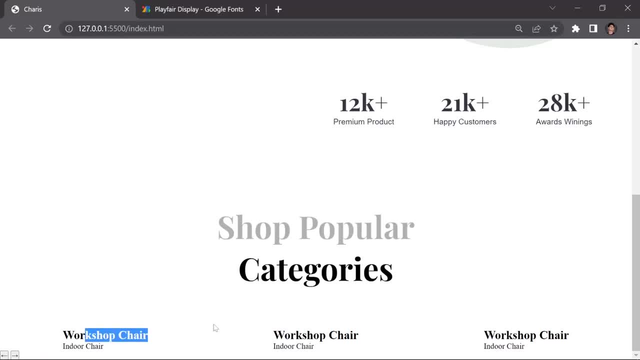 and align items. i'm going to set that to center and cell file and this is how to center and cell file. and this is how to center and cell file and this is how it looks like for now. okay, so you know, it looks like for now. okay, so you know. it looks like for now. okay, so you know, i'm going to just provide a height of. i'm going to just provide a height of. i'm going to just provide a height of like 100 vh in this case, if you save. like 100 vh in this case, if you save. 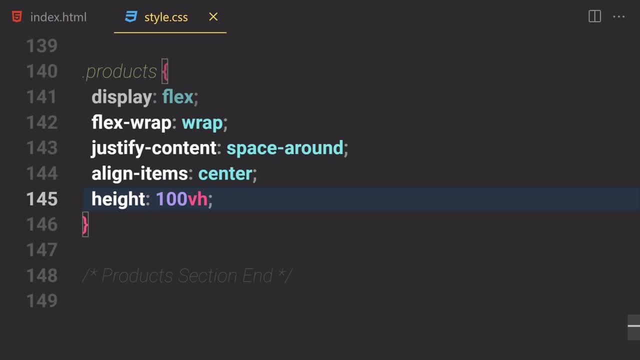 like 100 vh in this case. if you save that that, that this is how it looks like, so we will. this is how it looks like, so we will. this is how it looks like, so we will remove this 100 vh height from there. remove this 100 vh height from there. 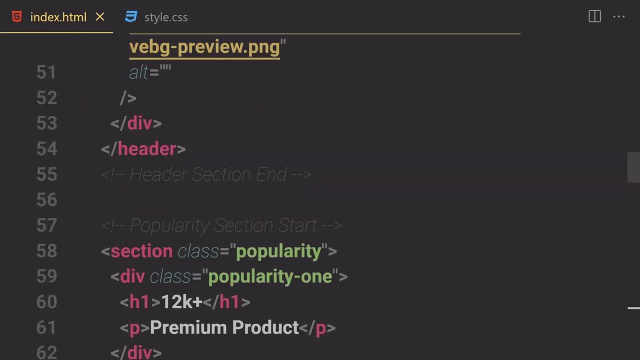 remove this 100 vh height from there just in a second. i just kind of want to, just in a second. i just kind of want to, just in a second. i just kind of want to show you everything, so let's just see. show you everything. so let's just see. 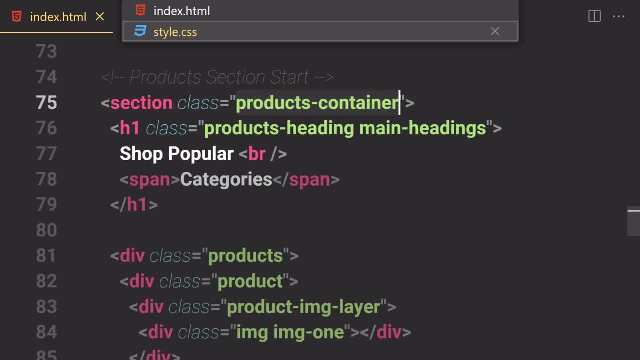 show you everything. so let's just see what will be the container- so products. what will be the container, so products. what will be the container, so products container. i'm going to copy that container, i'm going to copy that container, i'm going to copy that and i'm going to just paste it right here. 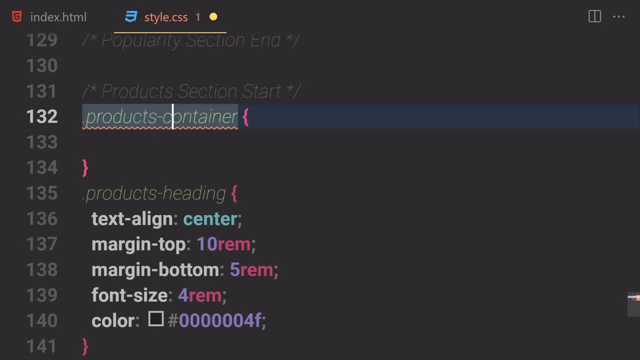 and i'm going to just paste it right here. and i'm going to just paste it right here: and let's just provide that heading. or, and let's just provide that heading, or, and let's just provide that heading, or, not having that height from there cut. 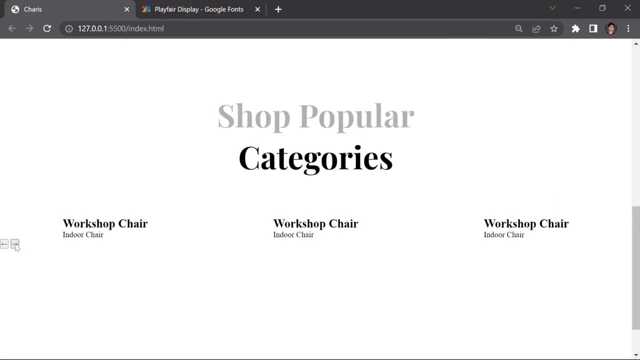 not having that height from there cut, not having that height from there, cut it from there and paste right here, and it from there and paste right here, and it from there and paste right here. and this is how currently things looks like. this is how currently things looks like. 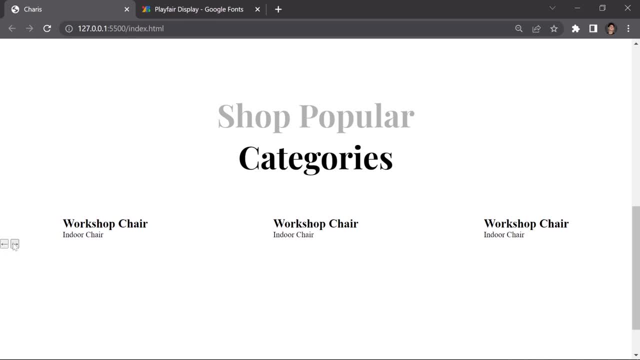 this is how currently things looks like. so we have these kind of two buttons, so we have these kind of two buttons. so we have these kind of two buttons right here, and we have two rows right here, and we have two rows right here and we have two rows- uh, or arrows, right here. 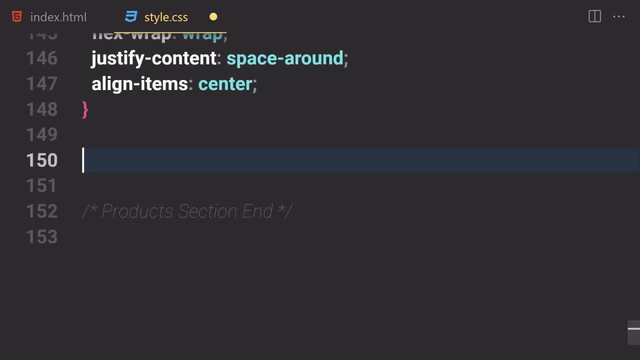 uh, or arrows right here, uh, or arrows right here, so anyways. so now let's just start, so anyways. so now let's just start. so anyways. so now let's just start working on over each product. so i'm going working on over each product. so i'm going. 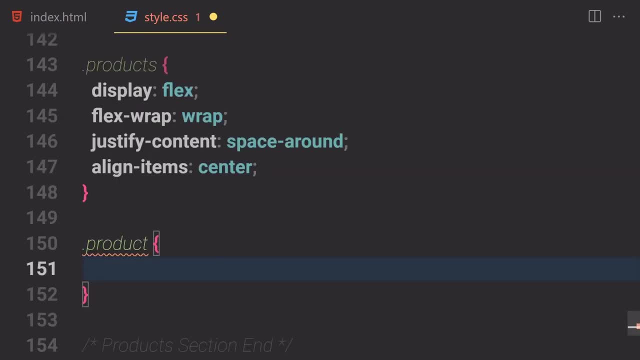 working on over each product, so i'm going to just select there first of all, to just select there first of all, to just select there first of all product. so that was a plural products product, so that was a plural products product, so that was a plural products and this is a product, right here, okay, 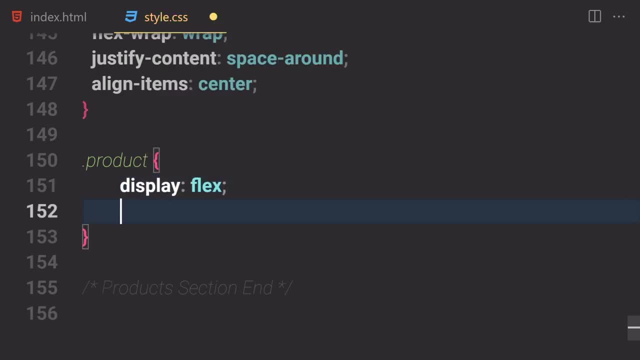 and this is a product right here, okay, and this is a product right here, okay, so let's just use our display flags. and so let's just use our display flags. and so let's just use our display flags. and uh, flex direction in this case will be. 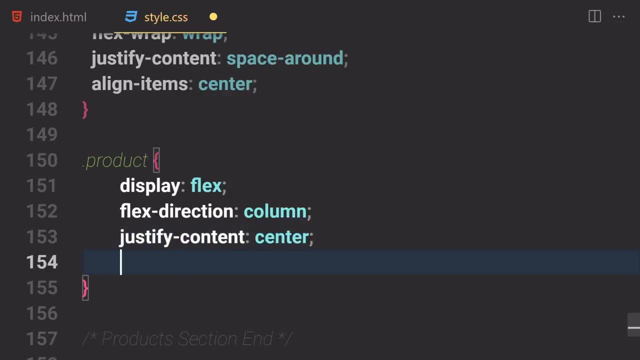 uh, flex direction in this case will be: uh. flex direction in this case will be: now set to column and justify content. now set to column and justify content. now set to column and justify content. i'm going to use like scenery align. i'm going to use like scenery align. 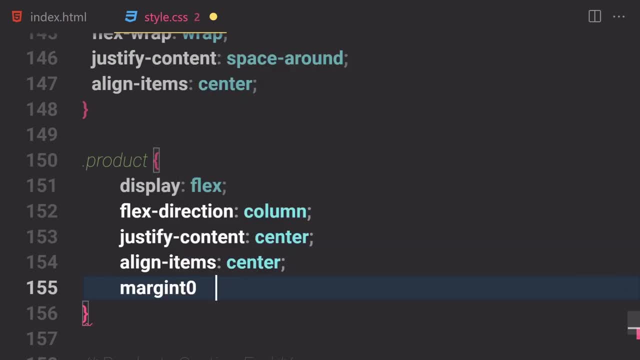 i'm going to use like scenery, align items. i'm going to also use center and items. i'm going to also use center and items. i'm going to also use center and margin for the top, margin for the top, margin for the top, uh, margin, top, if you just set to 50. 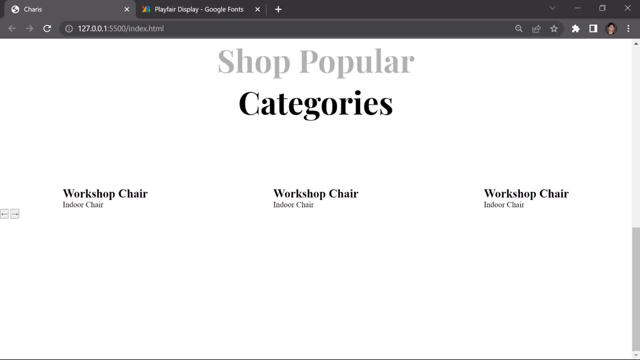 uh margin top if you just set to 50. uh margin top if you just set to 50 pixels. so if you sell a file and this pixels, so if you sell a file and this pixels, so if you sell a file, and this is how it looks like for now anyways, so 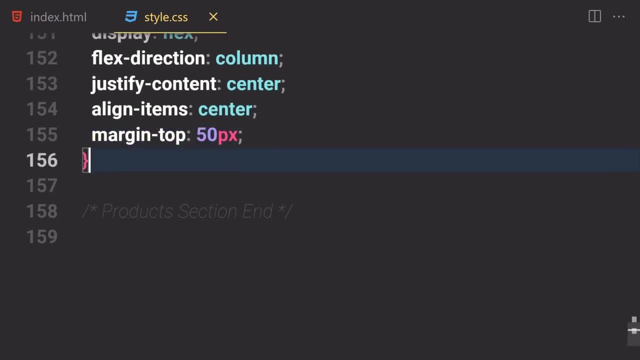 is how it looks like for now anyways. so is how it looks like for now anyways. so now, let's just start working on our. now, let's just start working on our. now, let's just start working on our product image layer. so i'm going to product image layer, so i'm going to 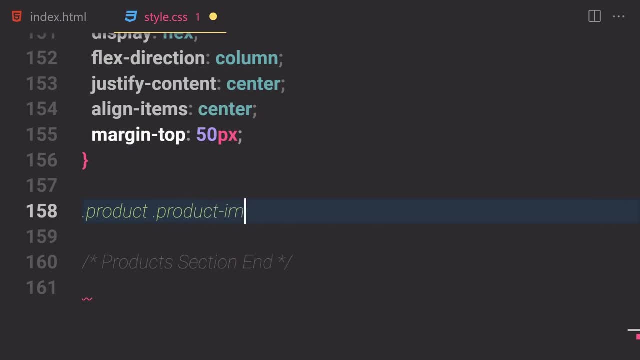 product image layer. so i'm going to first of all select my product and then first of all select my product and then first of all select my product, and then we have a product- uh- img and layer. okay, we have a product uh- img and layer. okay, we have a product- uh- img and layer- okay. so this class, let me just show you. 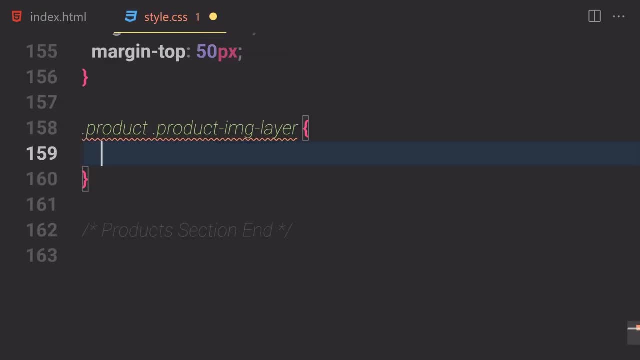 so this class, let me just show you. so this class, let me just show you. so we have this class for all of their. so we have this class for all of their. so we have this class for all of their layers. so i'm going to just provide a. 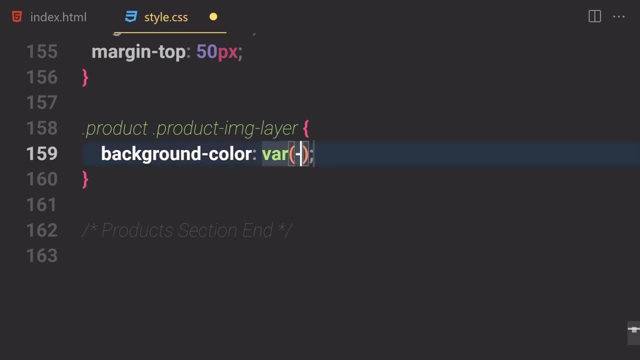 layers. so i'm going to just provide a layers, so i'm going to just provide a background color and now it will be set background color. and now it will be set background color and now it will be set to totally that main color which we, to totally that main color which we. 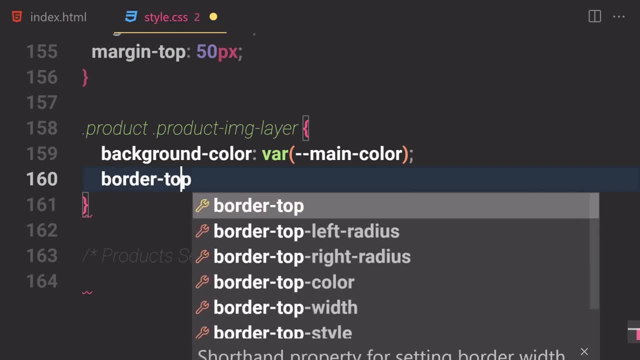 to totally that main color which we declare up above, declare up above, declare up above. and here we are going to be using a, and here we are going to be using a, and here we are going to be using a border for top left radius. i'm going to 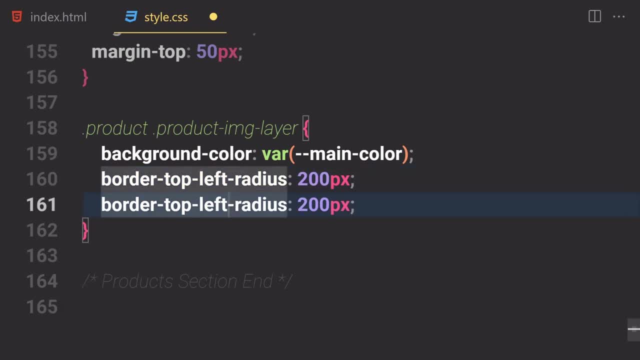 border for top left radius. i'm going to border for top left radius. i'm going to give like 200 pixel, duplicate that. one. give like 200 pixel, duplicate that one. give like 200 pixel, duplicate that one more time. and this is going to be it for. 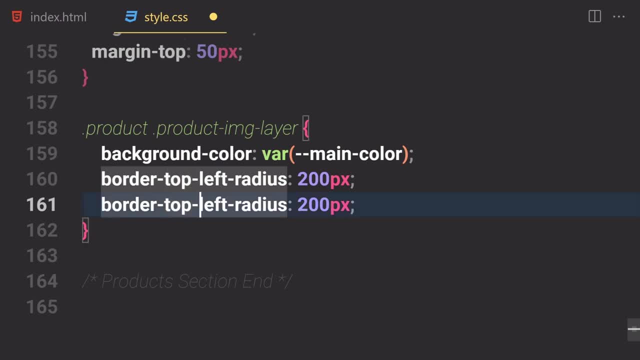 more time and this is going to be it for more time, and this is going to be it for the uh all right. so the uh all right, so the uh all right. so top left right and top top left right, top left right and top top left right. 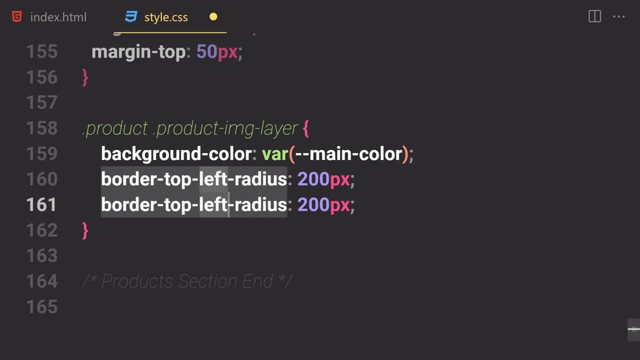 top left right and top top left right, uh, border top left radius, and then we uh border top left radius, and then we uh border top left radius, and then we have border right radius, there we go. so have border right radius, there we go. so have border right radius, there we go. so, padding, i'm going to give him like 20. 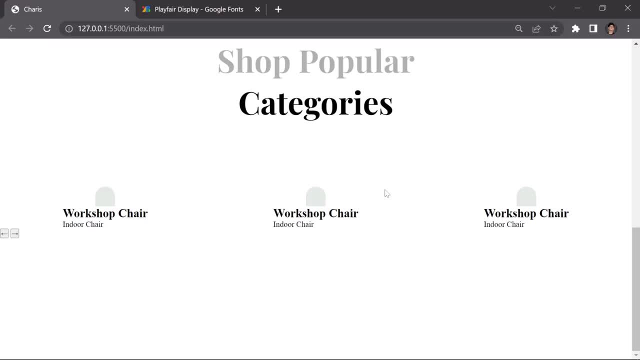 padding. i'm going to give him like 20 padding. i'm going to give him like 20 pixels if you sell that, and here you can pixels if you sell that, and here you can pixels if you sell that, and here you can see. this is how it looks like for now. 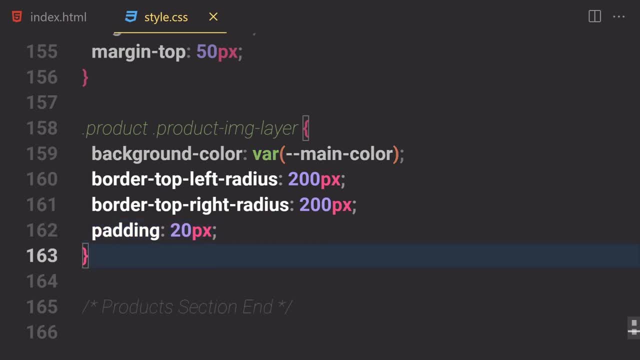 see, this is how it looks like for now. see, this is how it looks like for now anyway. so now let's just start working anyway. so now, let's just start working anyway. so now let's just start working on our image, and then you'll get to see. 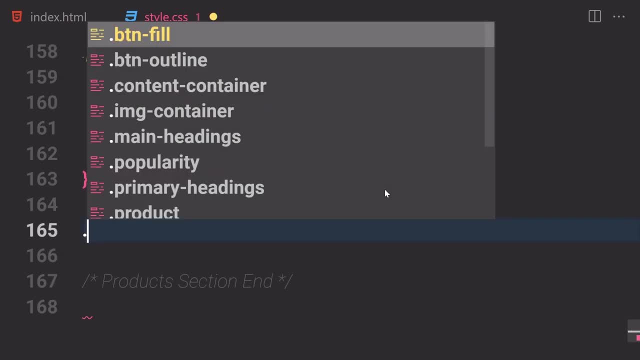 on our image and then you'll get to see on our image and then you'll get to see that will grow just a second. so first of that will grow just a second. so first of that will grow just a second. so first of all, let's just start working on our 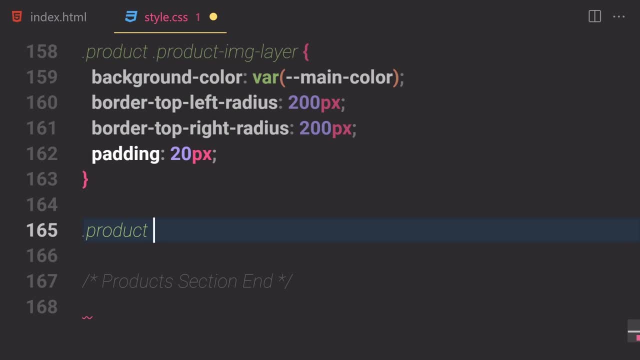 all. let's just start working on our all. let's just start working on our product. let's just select our product product. let's just select our product product. let's just select our product right here inside that product. we are right here inside that product, we are. 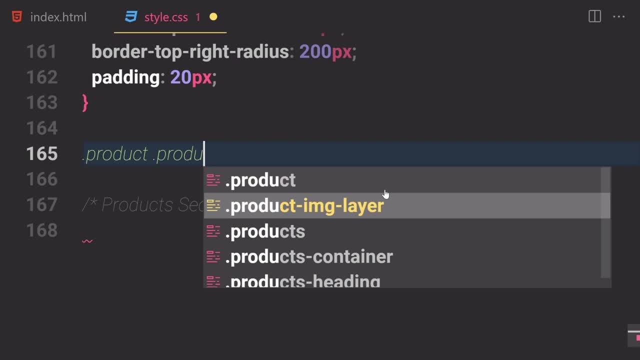 right here inside that product, we are going to be selecting our image layer. so going to be selecting our image layer. so going to be selecting our image layer, so product image layer, and now let's just product image layer. and now let's just product image layer, and now let's just select all of our images. so i'm going to 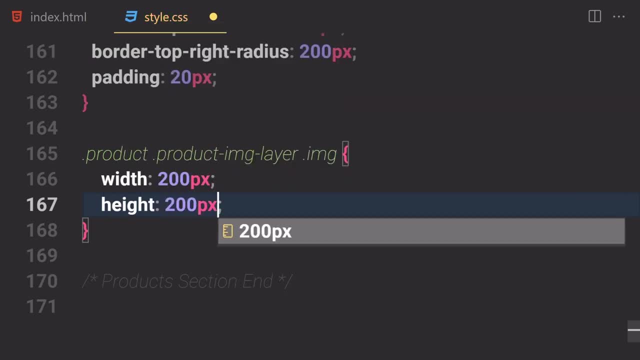 select all of our images. so i'm going to select all of our images, so i'm going to give them a width of like 200 pixel and give them a width of like 200 pixel, and give them a width of like 200 pixel, and height will be also set to 200 pixel. so 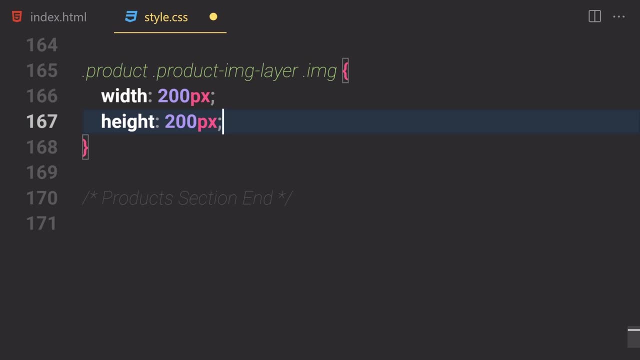 height will be also set to 200 pixel. so height will be also set to 200 pixel. so now, let's just apply new images for all. now, let's just apply new images for all. now, let's just apply new images for all, of their image one, image, two and image. 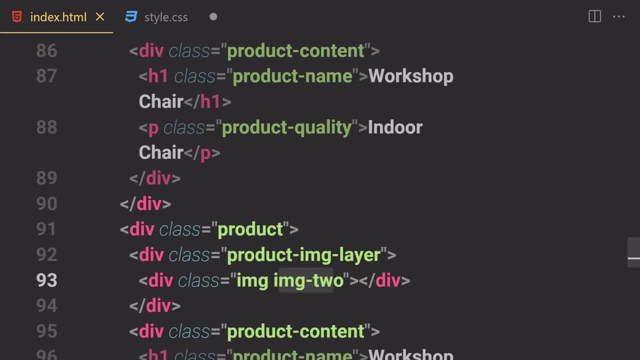 of their image one, image two, and image of their image one, image two and image three classes which we provide right, three classes which we provide right, three classes which we provide right here. so this is going to be image two here. so this is going to be image two. 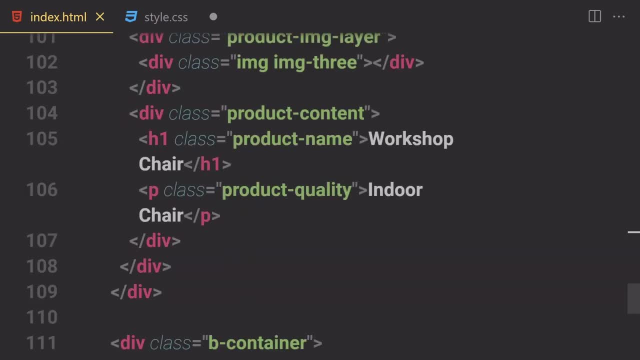 here. so this is going to be image two, and this is going to be image one, and, and this is going to be image one, and, and this is going to be image one, and that one is going to be the image three. that one is going to be the image three. 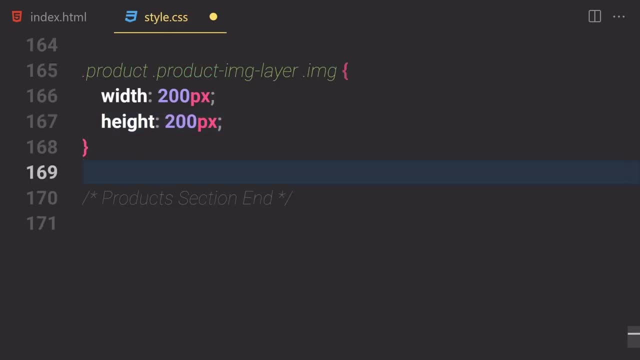 that one is going to be the image three, right here, anyways. so now, let's just right here anyways. so now, let's just right here anyways. so now let's just start working on that real quick. so what? start working on that real quick. so what, start working on that real quick? so what do we have to do? first of all, you know, do we have to do first of all? you know? do we have to do first of all, you know? i'm going to copy all of that selector. i'm going to copy all of that selector. i'm going to copy all of that selector from there. it's kind of long to write. 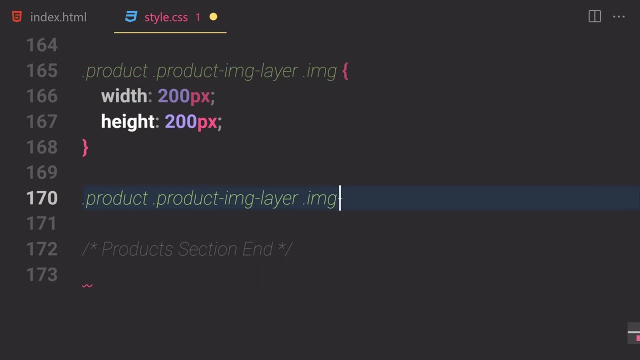 from there- it's kind of long to write from there, it's kind of long to write it- and i'm going to paste it right here, it and i'm going to paste it right here, it and i'm going to paste it right here. so, instead of writing img, so i'm going 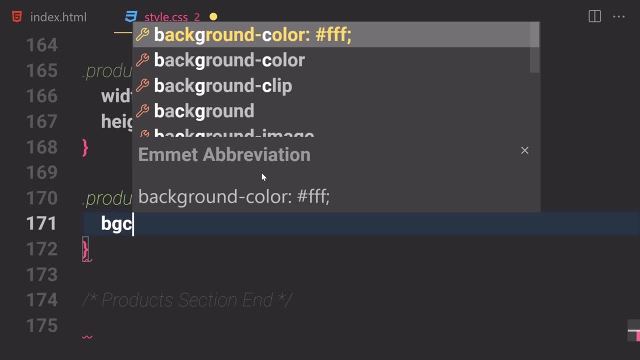 so instead of writing img, so i'm going. so, instead of writing img, so i'm going to just write img1 and let's just change to just write img1, and let's just change to just write img1, and let's just change the background to be: 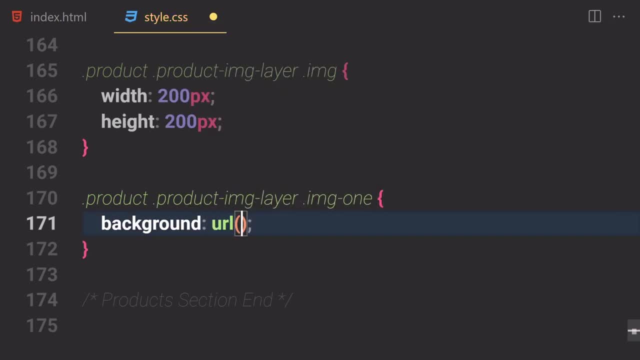 the background to be. the background to be not a color but just a background, not a color but just a background. not a color but just a background. shorthand, and i'm going to provide a url shorthand, and i'm going to provide a url shorthand and i'm going to provide a url of images. so i'm going to go to the. 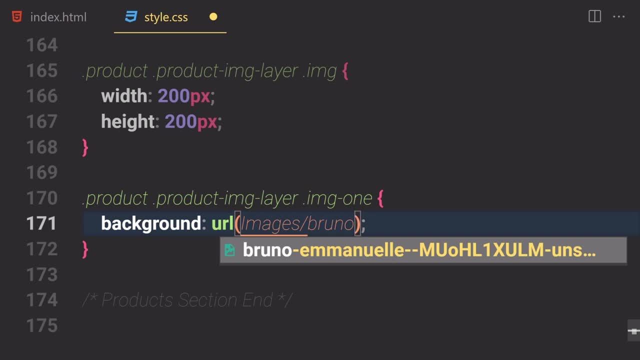 of images. so i'm going to go to the of images. so i'm going to go to the images and i'm going to also provide that images. and i'm going to also provide that images and i'm going to also provide that bruno, or whatever the name is, i'm going 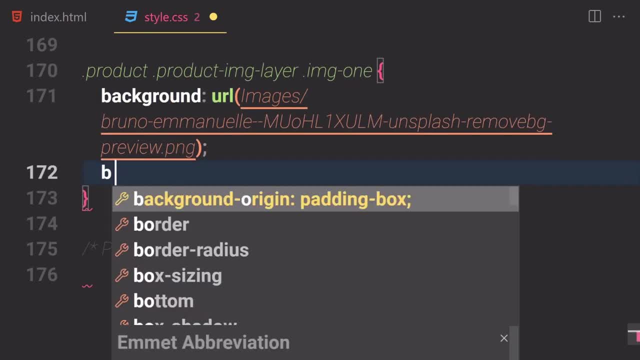 bruno or whatever the name is. i'm going, bruno or whatever the name is, i'm going to just select that image and i'm going to just select that image and i'm going to be providing a background size of, to be providing a background size of. 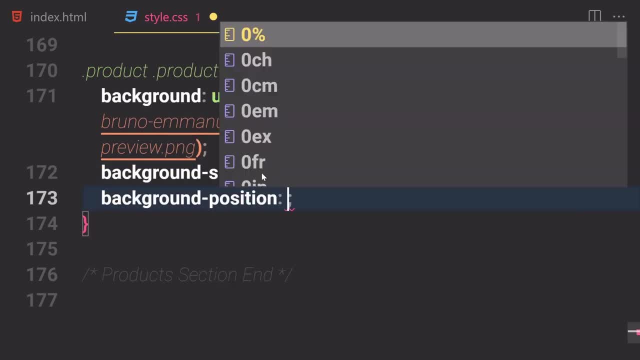 to be providing a background size of holy cover, and i'm going to also provide holy cover and i'm going to also provide holy cover and i'm going to also provide a background position, a background position, a background position of center, of center, of center not called, but center. okay, so let's just 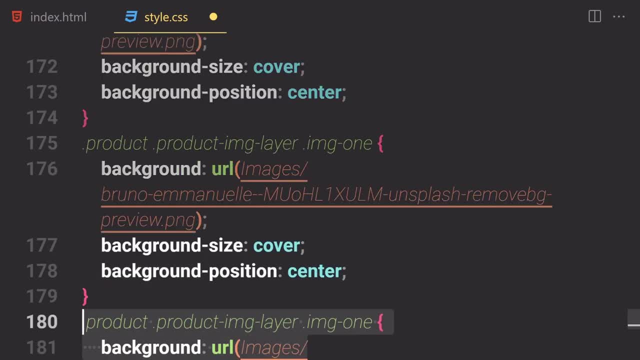 not called but center. okay, so let's just not called but center, okay, so let's just duplicate that two times so one and two, duplicate that two times so one and two, duplicate that two times so one and two, and this is going to be now it for image. 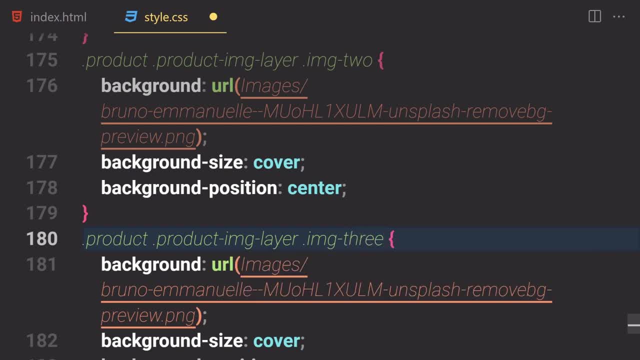 and this is going to be now it for image and this is going to be now it for image. second, one like two, and this is going to second one like two, and this is going to second one like two, and this is going to be the image three. okay, and now let's. 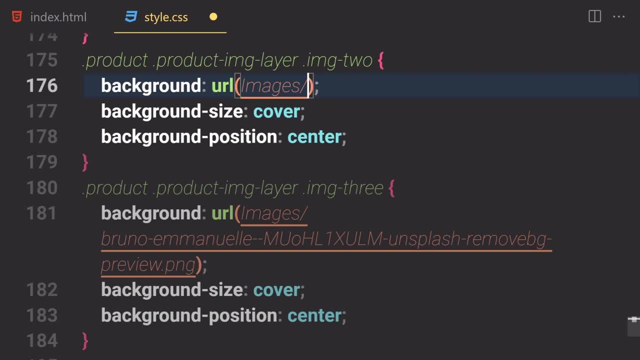 be the image three, okay, and now let's be the image three, okay, and now let's just reuse this. or you know what, let's just reuse this. or you know what, let's just reuse this. or you know what, let's just remove these images from there. so just remove these images from there. so just remove these images from there. so the second image i'm going to be the second image i'm going to be the second image i'm going to be selecting- is that you know what the selecting is, that you know what the 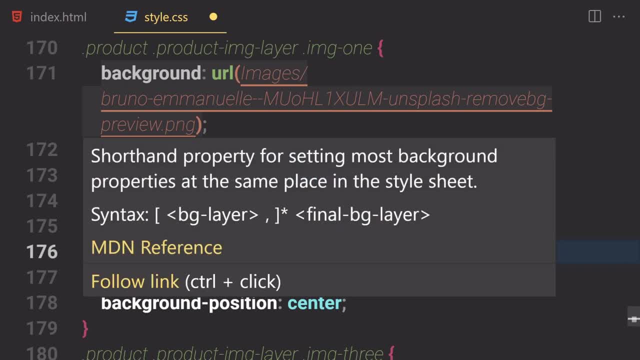 selecting is that you know what the first image will be for. first image will be for: first image will be for um daniels. so let's just remove um daniels. so let's just remove um daniels. so let's just remove, yeah, daniels, or whatever you want to. 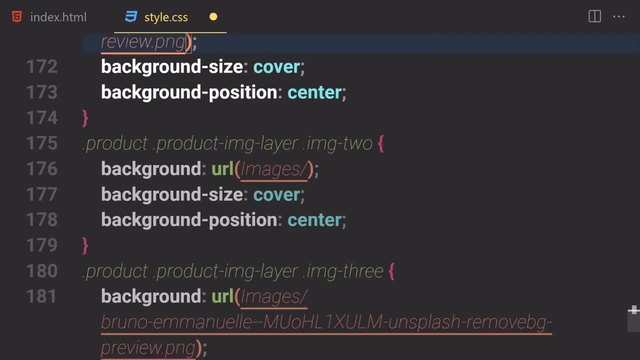 yeah, daniels, or whatever you want to. yeah, daniels, or whatever you want to call it. so i'm going to select that and call it. so i'm going to select that and call it. so i'm going to select that. and now let's just select our second image. 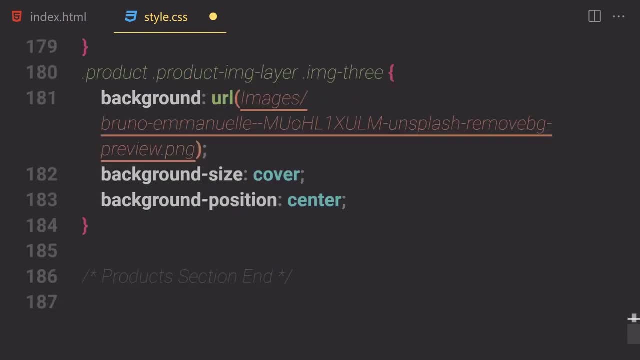 now let's just select our second image. now let's just select our second image and provide that bruno or whatever the, and provide that bruno or whatever the, and provide that bruno or whatever the guy name is, guy name is, guy name is. and then we have a scott. so let's just 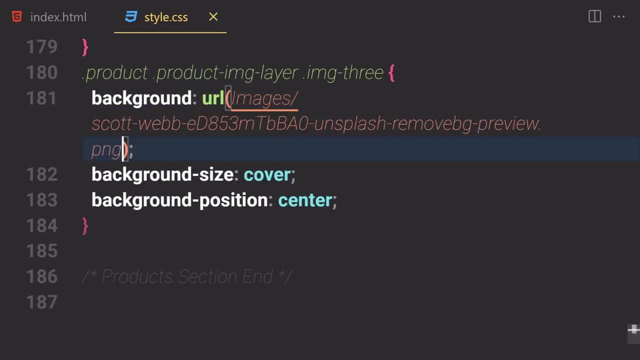 and then we have a scott, so let's just: and then we have a scott, so let's just remove that, remove that, remove that and write a scott. and now, if you save and write a scott, and now if you save and write a scott, and now if you save that, and this is how it looks like for 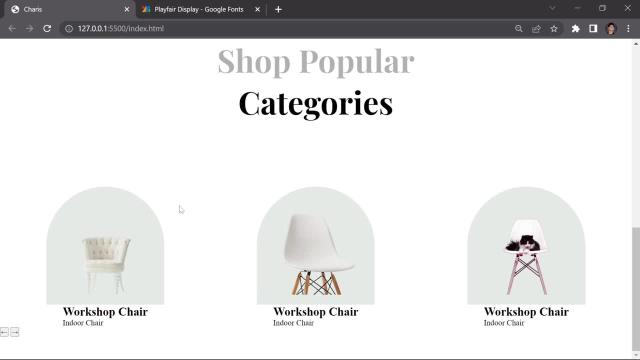 that, and this is how it looks like for that, and this is how it looks like for now. okay, so everything is looking now. okay, so everything is looking now. okay. so everything is looking perfect in the way i expect them to be, perfect, in the way i expect them to be. 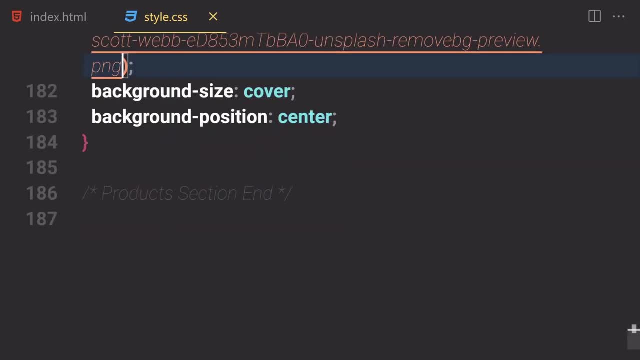 perfect in the way i expect them to be looking. so now let's just take care of looking. so now, let's just take care of looking. so now let's just take care of all these other stuff right here. so all these other stuff right here, so all these other stuff right here. so what do we have to do? let's just start. 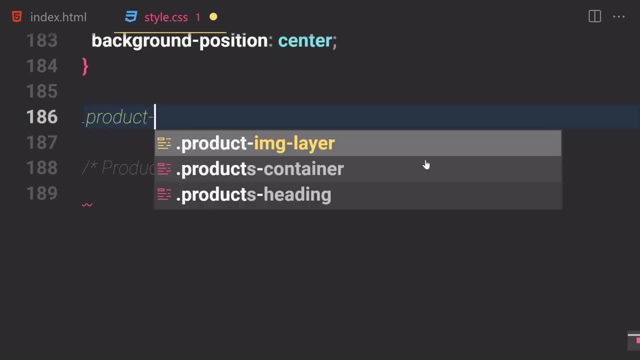 what do we have to do? let's just start. what do we have to do? let's just start working on our products- uh content. so we working on our products, uh content, so we working on our products, uh content, so we have product content so like. so i'm. 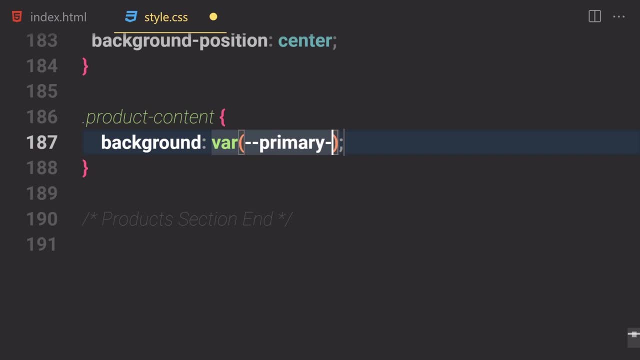 have product content, so like. so i'm have product content, so like. so i'm gonna write a background color of gonna write a background color, of gonna write a background color of totally one of primary color. okay, so, totally one of primary color. okay, so, totally one of primary color. okay, so let's just provide a padding of like 27. 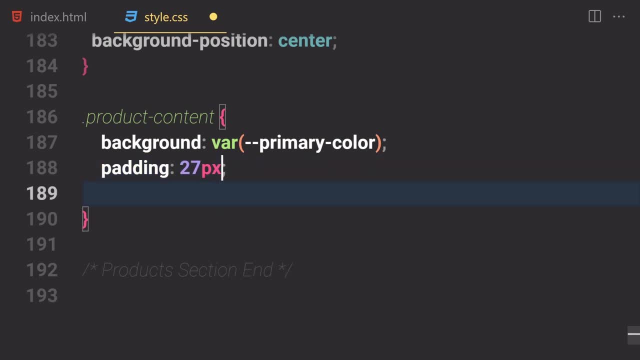 let's just provide a padding of like 27. let's just provide a padding of like 27 would be fine, so 27 would be fine, so 27 would be fine, so 27 pixel, pixel, pixel. and also the padding for the bottom i'm. and also the padding for the bottom i'm. 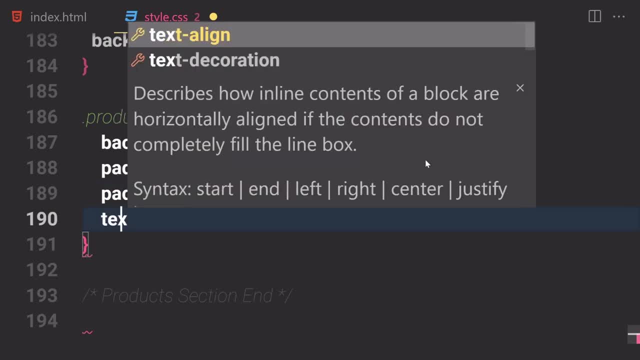 and also the padding for the bottom. i'm going to provide like padding bottom of. going to provide like padding bottom of. going to provide like padding bottom of 50 pixel and text alignment: i'm going to 50 pixel and text alignment: i'm going to 50 pixel and text alignment: i'm going to set that to center and color will be now. 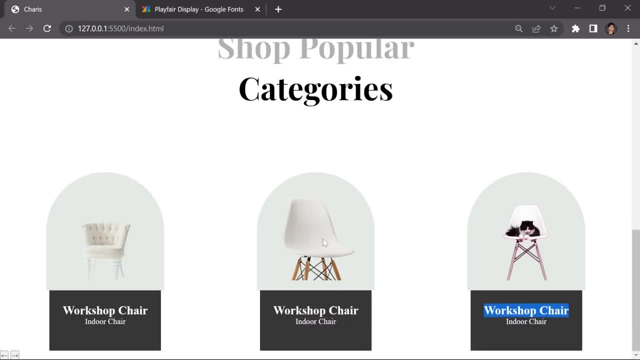 set that to center and color will be now. set that to center and color will be now totally white. so if you save that and totally white, so if you save that and totally white, so if you save that and this is how it looks like, okay. so if this is how it looks like okay. so, if this is how it looks like, okay. so if you zoom in a bit, you zoom in a bit, you zoom in a bit, all right. so i guess we have to provide. all right, so i guess we have to provide. 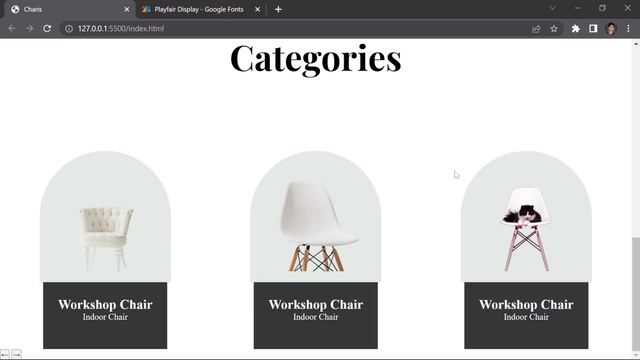 all right. so i guess we have to provide a little bit of spacing in there, a little bit of spacing in there, a little bit of spacing in there, and then it will look a bit fine. and then it will look a bit fine, and then it will look a bit fine, or we can just run down the images, or 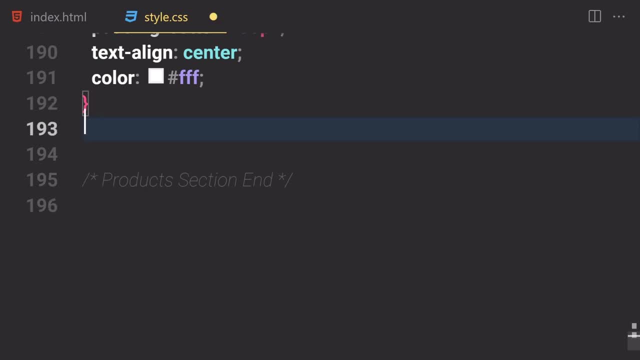 or we can just run down the images, or. or we can just run down the images or not of images by the font size, not of images by the font size, not of images by the font size. let's just select their product name. let's just select their product name. 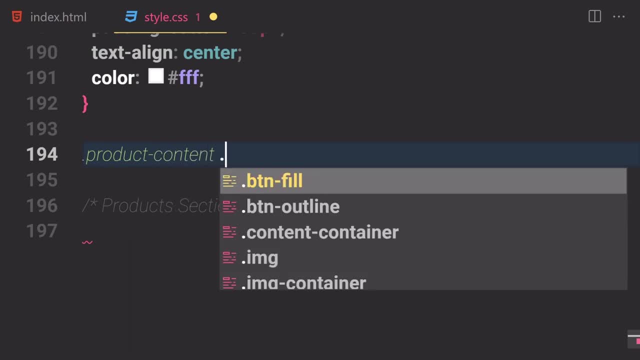 let's just select their product name first of all. i'm going to use a product. first of all. i'm going to use a product. first of all, i'm going to use a product content inside this product content. we content inside this product content. we content inside this product content. we want to select our product. 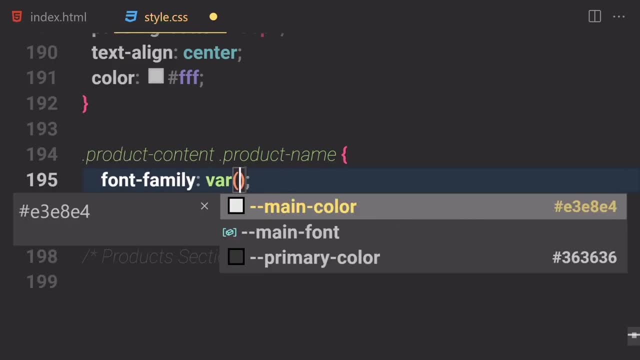 want to select our product? want to select our product? uh name, okay. so i'm going to just uh name. okay, so i'm going to just uh name. okay. so i'm going to just provide a font family of that, provide a font family of that, provide a font family of that, not war, but sans serif and margin for. 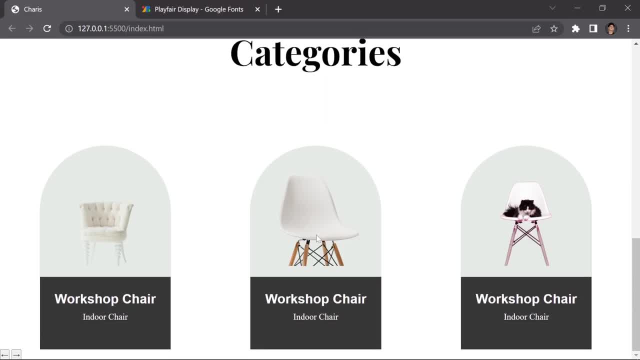 not war but sans serif and margin for not war but sans serif and margin for the bottom. i'm going to provide like 10, the bottom. i'm going to provide like 10, the bottom. i'm going to provide like 10 pixels. so if you sell that and this is, 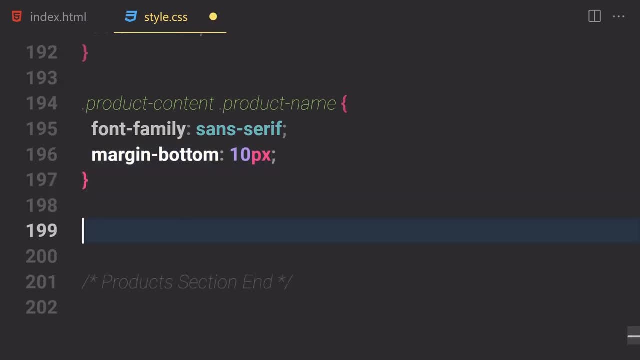 pixels. so if you sell that and this is pixels. so if you sell that and this is how it looks like right now, okay, so it's how it looks like right now. okay, so it's how it looks like right now. okay, so it's kind of a increase a bit. now let's just 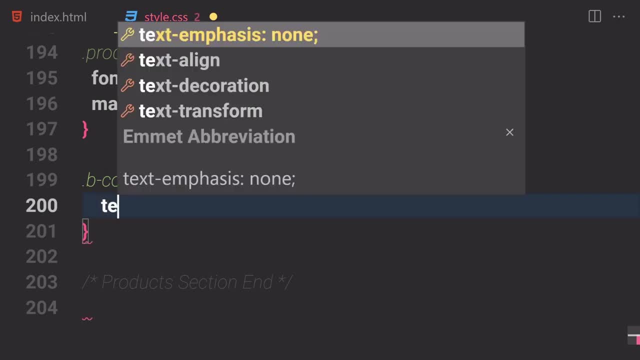 kind of a increase a bit now. let's just kind of a increase a bit now. let's just select order b- container or buttons. select order b- container or buttons. select order b- container or buttons. container and text alignment will be now. container and text alignment will be now. 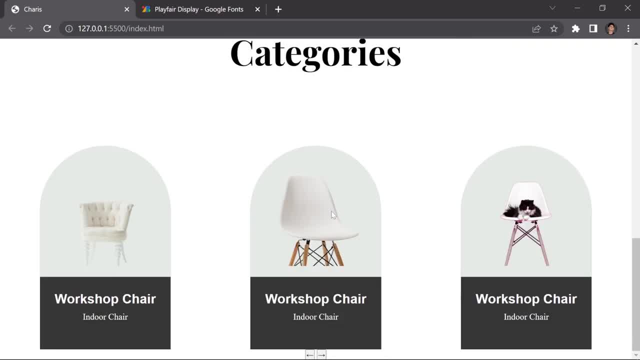 container and text alignment will be now set to center. so if you sell that, it set to center. so if you sell that, it set to center. so if you sell that, it will push that buttons to the bottom. you will push that buttons to the bottom. you will push that buttons to the bottom. you know i'm going to remove that height. 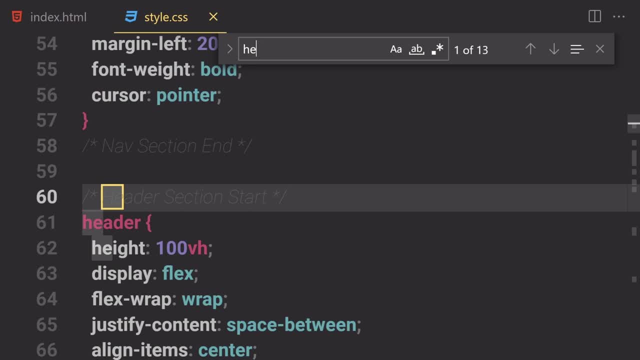 know i'm going to remove that height. know i'm going to remove that height from there. you don't need it anymore. so from there, you don't need it anymore. so from there, you don't need it anymore. so high of 100 vh. so i'm going to remove. 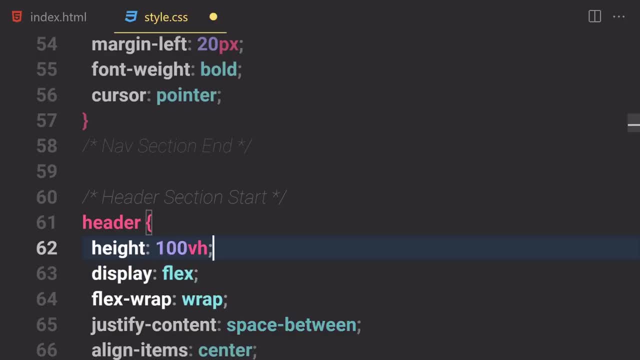 high of 100 vh. so i'm going to remove high of 100 vh. so i'm going to remove that cell file. or you know what, not that? that cell file. or you know what, not that that cell file. or you know what, not that one. come on, man. 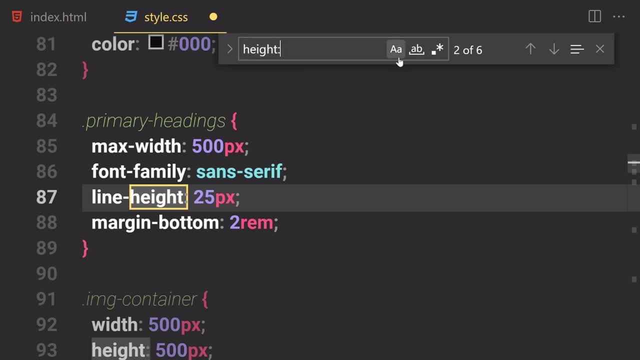 one. come on man. one come on man. uh selected one more time. uh selected one more time. uh selected one more time. height of 100 vh. height of 100 vh. height of 100 vh. uh, all right, so this is the first one. uh, all right, so this is the first one. 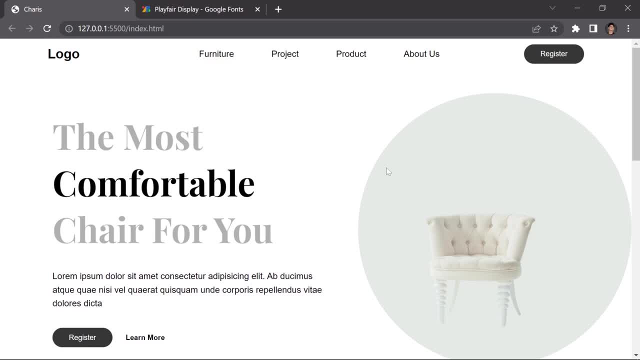 uh, all right, so this is the first one, this is the second one. so let's just, this is the first one, this is the second one. so let's just, this is the first one, this is the second one. so let's just remove that, remove that, remove that seven and yeah, that's looking fine. 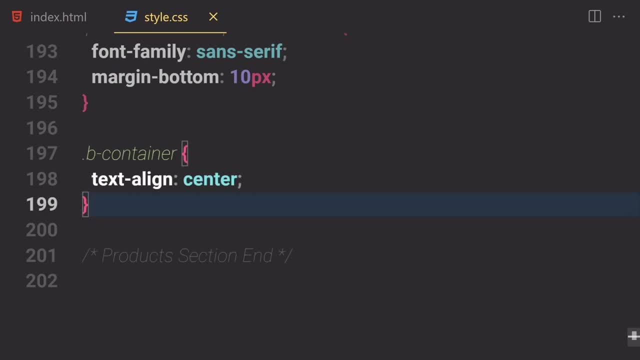 seven and yeah, that's looking fine. seven and yeah, that's looking fine. so that's there now. what else do you have to? that's there now. what else do you have to? that's there now. what else do you have to do? we have to select the b. 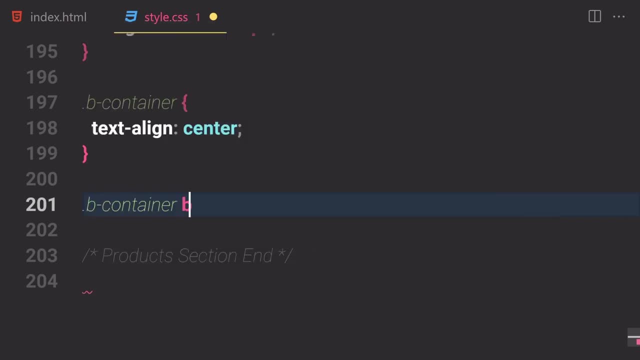 do we have to select the b? do we have to select the b and not just buttons, but just b? and and not just buttons, but just b? and, and not just buttons, but just b and container. and we want to select both of container and we want to select both of. 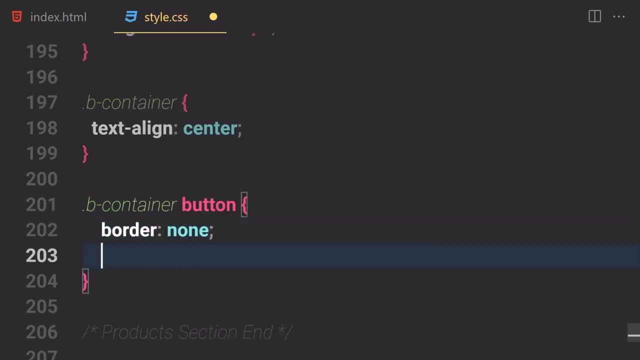 container and we want to select both of those buttons. i'm going to remove their those buttons. i'm going to remove their those buttons. i'm going to remove their border set that to none and also the border set that to none and also the border set that to none, and also the background will be transparent in this. 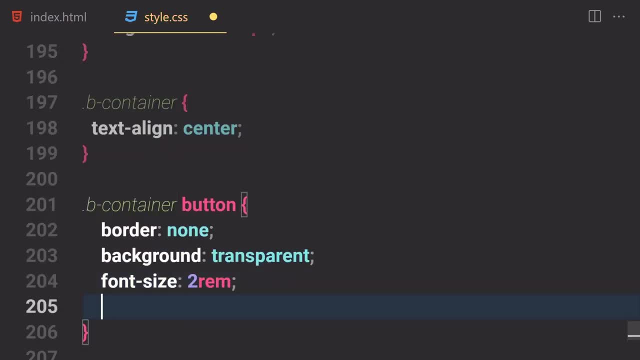 background will be transparent in this. background will be transparent in this case. and the font size: i'm going to case and the font size i'm going to case. and the font size i'm going to increase that to 2 ram and cursor will increase that to 2 ram and cursor will. 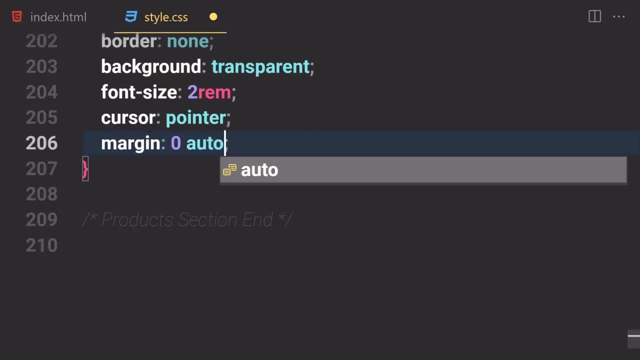 increase that to 2 ram and cursor will be pointer, be pointer, be pointer. i'm going to give a margin of zero auto. i'm going to give a margin of zero auto. i'm going to give a margin of zero auto and margin for the left will be set to. 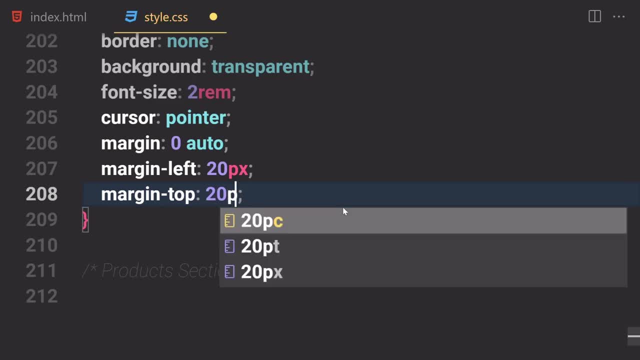 and margin for the left will be set to and margin for the left will be set to 20 pixel and margin: 20 pixel and margin: 20 pixel and margin: uh margin for the top, i'm gonna set uh margin for the top, i'm gonna set. 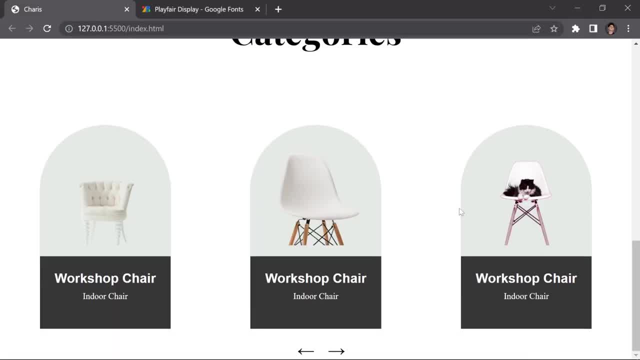 uh, margin for the top. i'm gonna set that to 10 pixels, if you saw that, and that to 10 pixels if you saw that, and that to 10 pixels, if you saw that. and this is how it looks like i guess you. this is how it looks like i guess you. 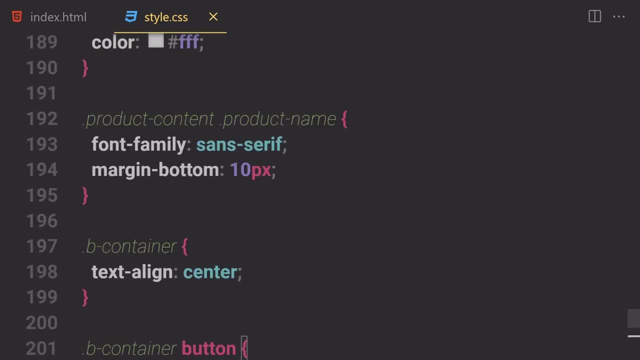 this is how it looks like. i guess you cannot see there. let me just show you cannot see there. let me just show you cannot see there. let me just show you that real quick, that real quick, that real quick. uh, okay, so we have product name, we have 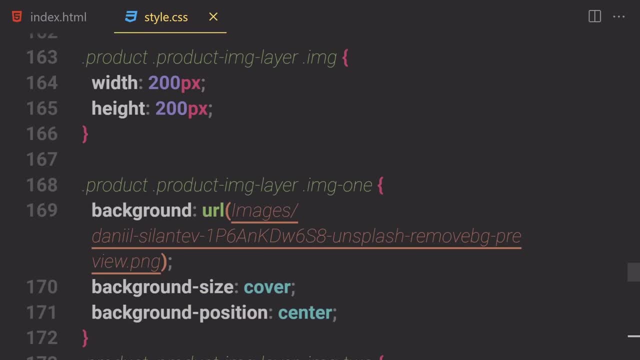 uh okay, so we have product name. we have. uh okay, so we have product name. we have a product blah blah blah, a product blah blah blah, a product blah blah blah. hmm, let's just provide a heart to none. hmm, let's just provide a heart to none. 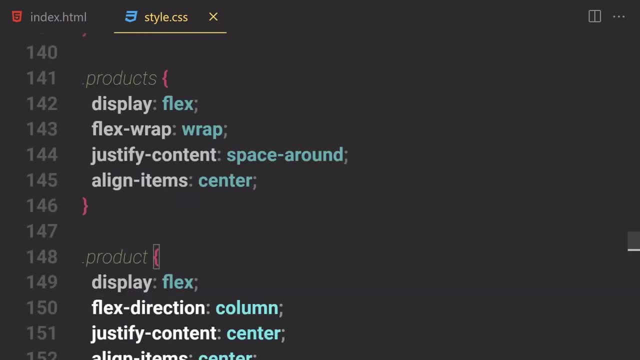 hmm, let's just provide a heart to none of the images, not the layers, but i guess of the images, not the layers, but i guess of the images, not the layers. but i guess to the product would be fine, to the product would be fine, to the product would be fine, or products would be fine. i'm going to. 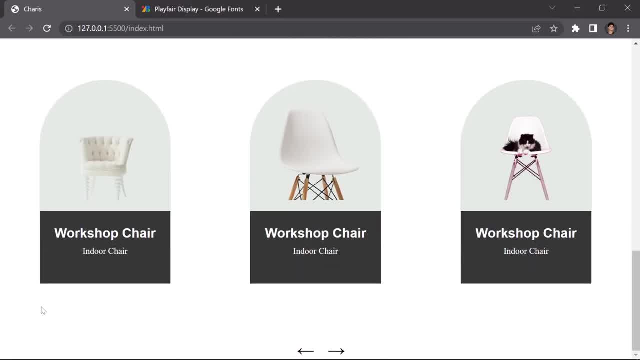 or products would be fine. i'm going to or products would be fine. i'm going to provide a height of 100 vh in there. if provide a height of 100 vh in there. if provide a height of 100 vh in there. if you save that. 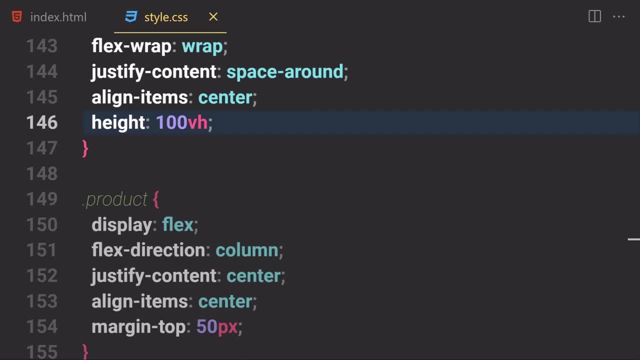 you save that, you save that, and you cannot see those buttons but, and you cannot see those buttons but, and you cannot see those buttons, but you will see that just in a second. you will see that just in a second. you will see that just in a second. anyways, i'm going to remove that height. 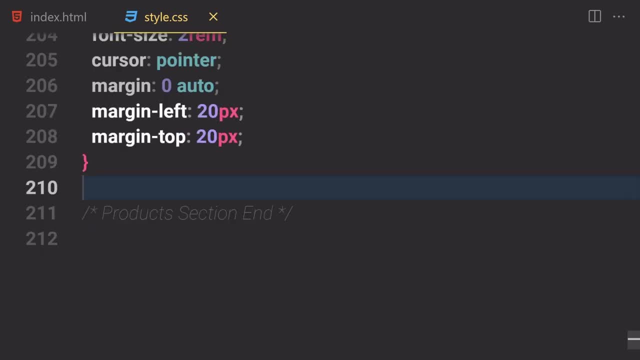 anyways, i'm going to remove that height. anyways, i'm going to remove that height from there and we are totally done with from there and we are totally done with from there and we are totally done with or um, whatever you call it, or product. or um, whatever you call it, or product. 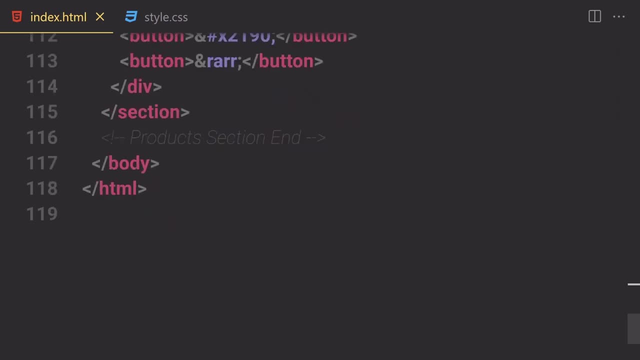 or, um, whatever you call it- or product section. now, let's jump into a new section. now let's jump into a new section. now let's jump into a new section called why choose us or why us section called why choose us or why us section called why choose us or why us. let me just write a comment for myself. 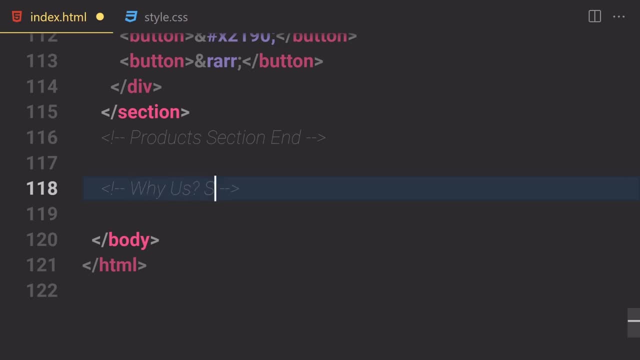 let me just write a comment for myself. let me just write a comment for myself: like: uh, why us question mark section? like uh, why us question mark section? like uh, why us question mark section start and then duplicate and section start and then duplicate and section start and then duplicate and section end. okay, so first of all, i'm going to 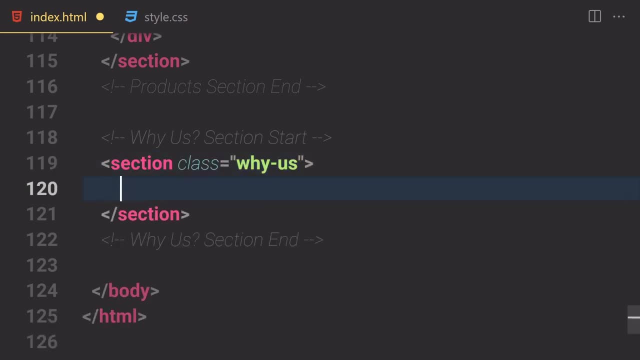 end, okay. so first of all, i'm going to end okay. so first of all, i'm going to just create a section with a class of, just create a section with a class of, just create a section with a class of y us. inside this section, we are going to 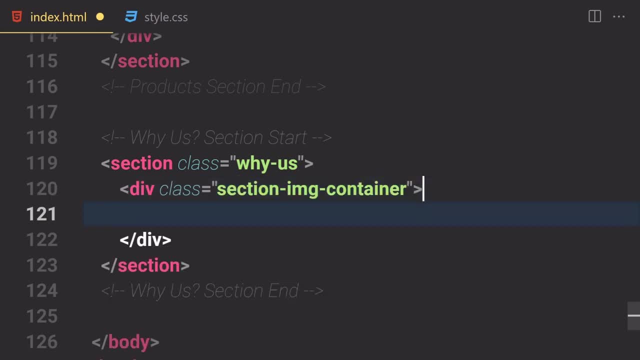 y us inside this section. we are going to y us inside this section. we are going to be using a div with a class of section. be using a div with a class of section. be using a div with a class of section, img and container inside. there we are. 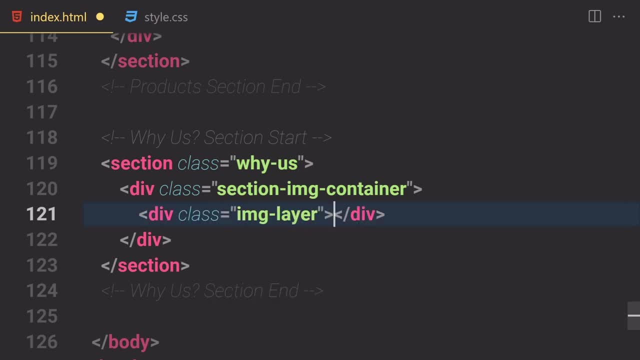 img and container inside there. we are img and container inside there. we are going to be creating a new div with a, going to be creating a new div with a, going to be creating a new div with a class of image layer and inside that we class of image layer and inside that we. 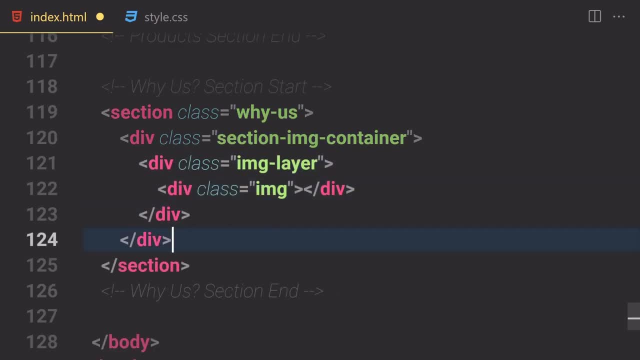 class of image layer and inside that, we are going to be just specifying one, are going to be just specifying one, are going to be just specifying one image. okay, so outside from all of these image. okay, so outside from all of these image. okay, so, outside from all of these div. but inside this section we're going 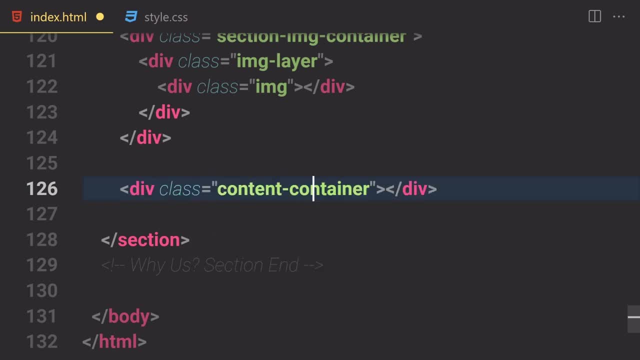 div, but inside this section we're going div, but inside this section we're going to be creating a new div with a class of. to be creating a new div with a class of. to be creating a new div with a class of content container inside this content. 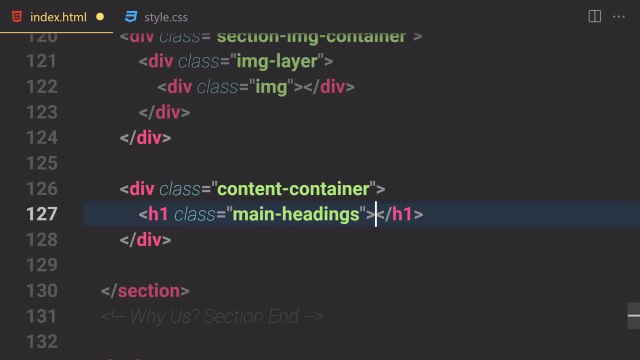 content container. inside this content content container, inside this content container, we are going to be using h1 container. we are going to be using h1 container. we are going to be using h1 with a class of main headings, with a class of main headings, with a class of main headings, and let's just probably like y choose. 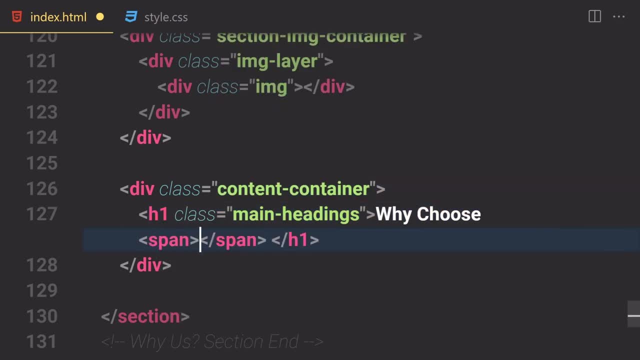 and let's just probably like y choose, and let's just probably like y choose: uh, yeah, that would be fine. and now let's uh: yeah, that would be fine. and now let's uh: yeah, that would be fine. and now let's just provide a span in here with no. 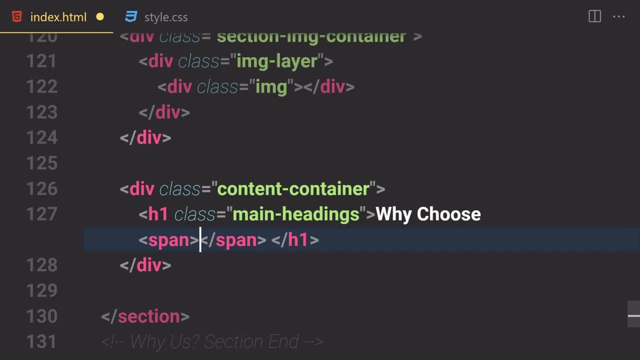 just provide a span in here with no, just provide a span in here with no classes, nothing inside there. classes, nothing inside there. classes, nothing inside there. but i'm going to just put like us in, but i'm going to just put like us in, but i'm going to just put like us in here. so ask and question mark and 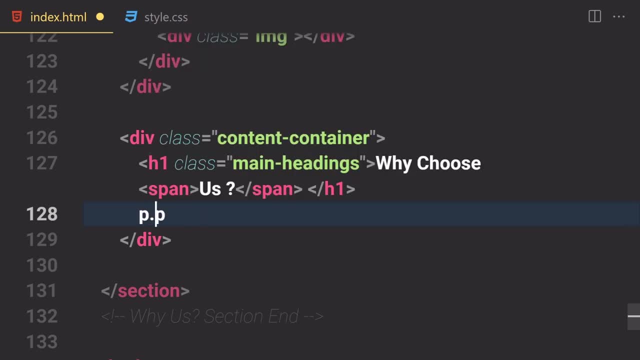 here so ask and question mark. and here, so ask and question mark. and underneath this, uh h1, what do we have to? underneath this, uh h1, what do we have to underneath this, uh h1? what do we have to do? i'm going to just write up, so i'm 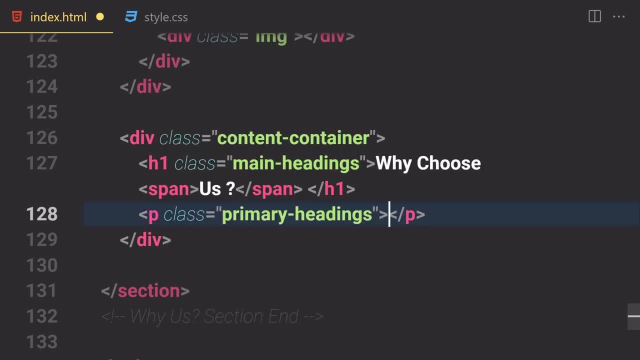 do i'm going to just write up. so i'm do, i'm going to just write up. so i'm going to provide a primary, going to provide a primary, going to provide a primary headings. so we are now reusing that headings. so we are now reusing that. 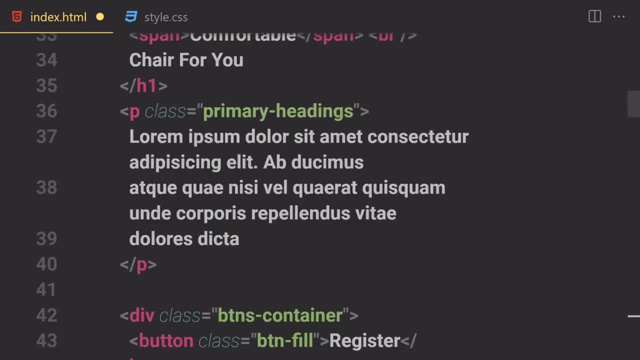 headings. so we are now reusing that class. so let's just copy that content class. so let's just copy that content class. so let's just copy that content from here as well, from here as well, from here as well. uh, yeah, i'm gonna copy all of that. 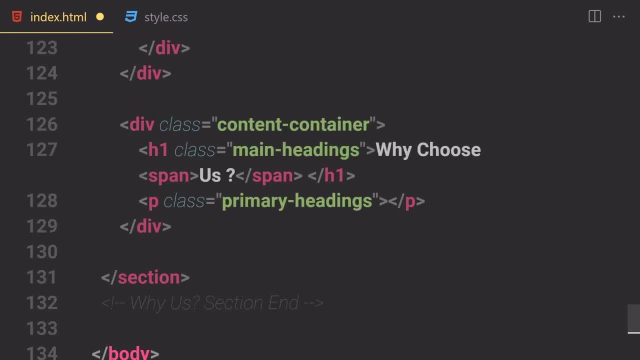 uh, yeah, i'm gonna copy all of that. uh, yeah, i'm gonna copy all of that content, so content, so content. so go to the bottom and i'm gonna paste. go to the bottom and i'm gonna paste. go to the bottom and i'm gonna paste inside this primary headings right here. 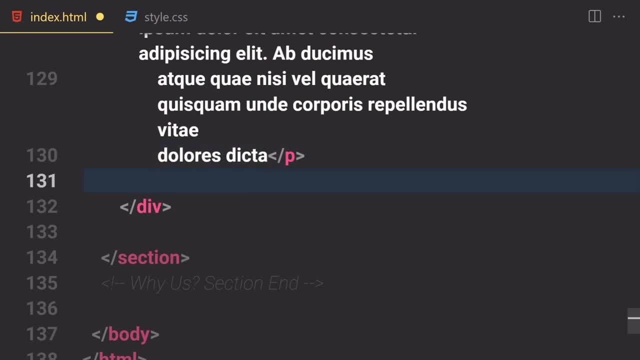 inside this primary headings, right here. inside this primary headings, right here. so outside from this paragraph, what do we so outside from this paragraph? what do we so outside from this paragraph? what do we have to do? have to do, have to do. uh, i'm gonna create a new div with a. 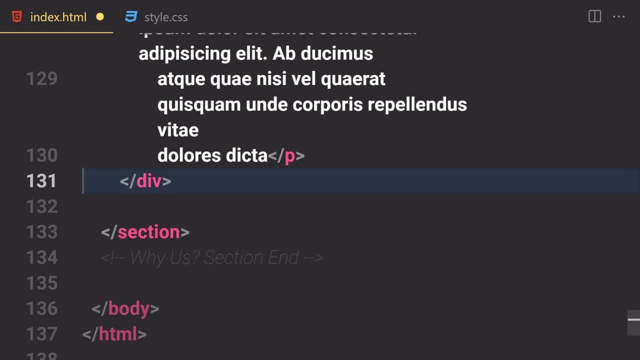 uh, i'm gonna create a new div with a. uh, i'm gonna create a new div with a class of you know what outside from this class of you know what outside from this class of you know what outside from this div event. so div event, so div event. so, uh, i'm gonna create a new paragraph, but 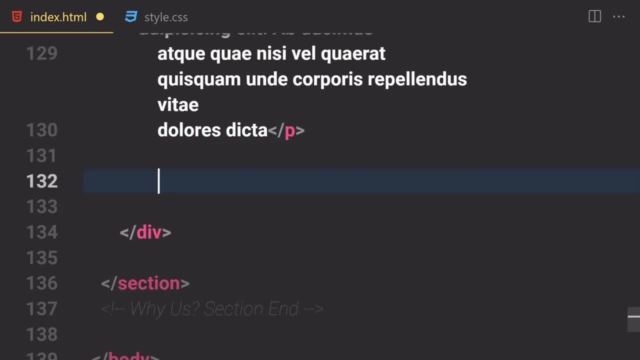 uh, i'm gonna create a new paragraph, but, uh, i'm gonna create a new paragraph, but not out, not out, not out. you know what? outside from this, you know what? outside from this, you know what? outside from this paragraph, i'm going to create a new div. 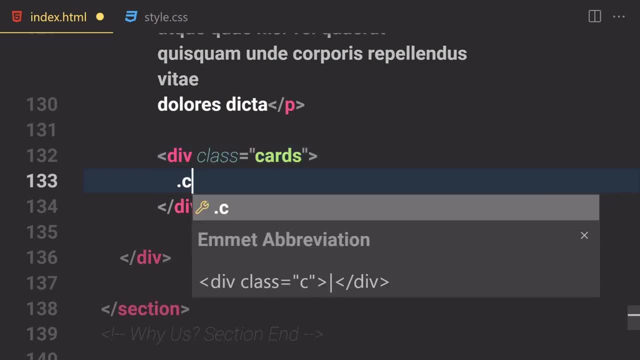 paragraph. i'm going to create a new div paragraph. i'm going to create a new div with a class of cards and sign these with a class of cards and sign these with a class of cards and sign these cards. we are going to be creating a card. 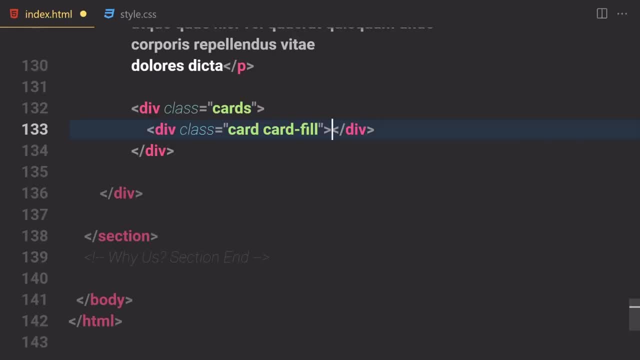 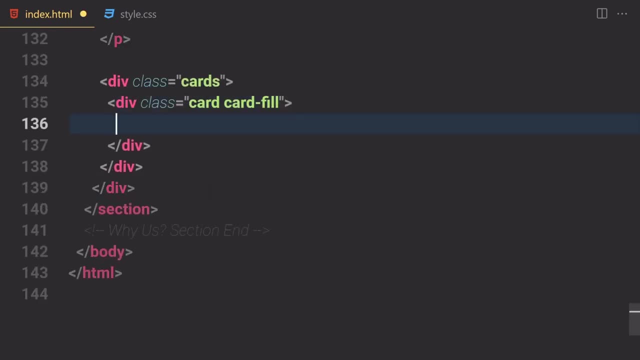 cards. we are going to be creating a card cards. we are going to be creating a card placing or html entity in here. so we have placing or html entity in here. so we have placing or html entity in here. so we have an symbol first of all, an symbol first of all. 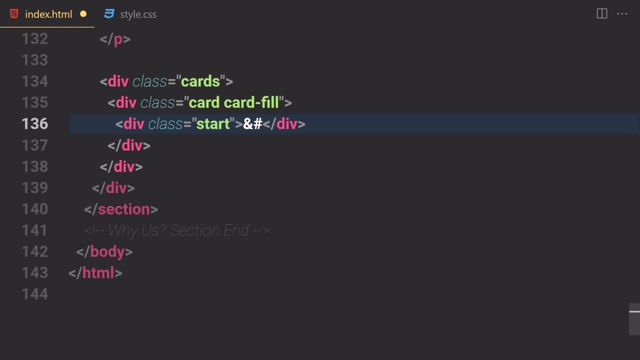 an symbol, first of all. uh, yeah and symbol. uh, yeah and symbol, uh, yeah and symbol. then we have a pound symbol, and then we, then we have a pound symbol, and then we, then we have a pound symbol, and then we have nine, seven, have nine, seven, have nine, seven, three, three, and now let's just close that. 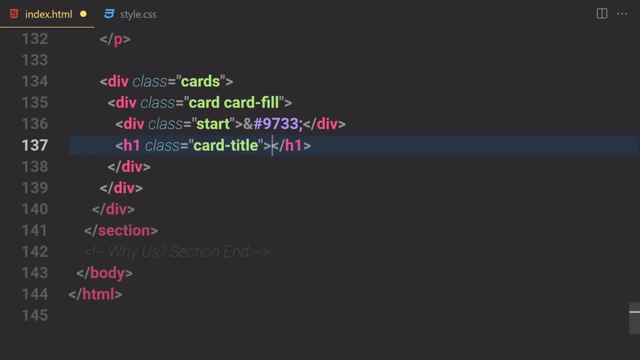 three and now let's just close that three. and now let's just close that. let's just write h1 with the class of. let's just write h1 with the class of. let's just write h1 with the class of card title. let's just put our title in. 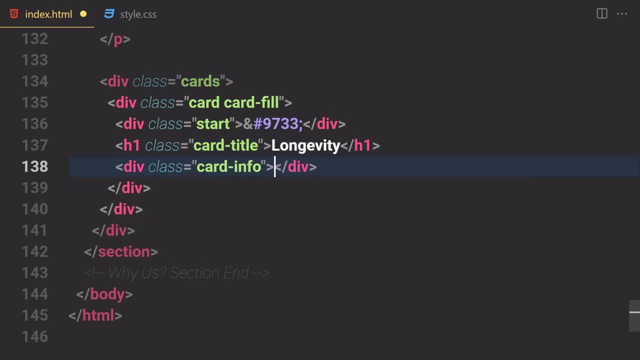 card title. let's just put our title in card title. let's just put our title in there and write a paragraph for card there. and write a paragraph for card there and write a paragraph for card info, info, info. this is going to be the paragraph, not a. 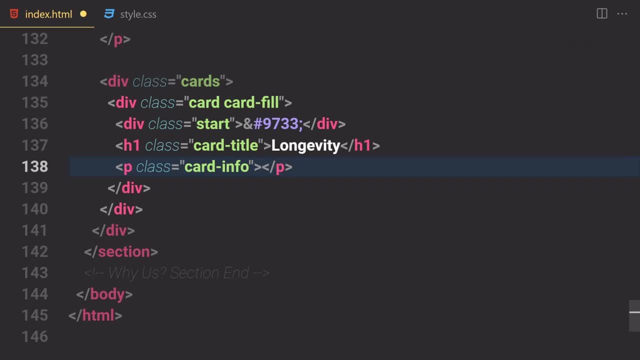 this is going to be the paragraph, not a. this is going to be the paragraph, not a div. so let's just change that to div. so let's just change that to div. so let's just change that to paragraph, paragraph, paragraph. and yeah, i'm going to paste that lorem. 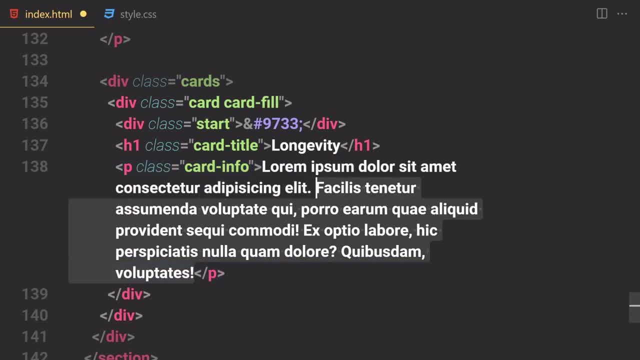 and yeah, i'm going to paste that lorem and yeah, i'm going to paste that lorem. lorem off a few lines, not that much. lorem off a few lines, not that much. lorem off a few lines, not that much. uh, elite would be fine so. uh, elite would be fine so. 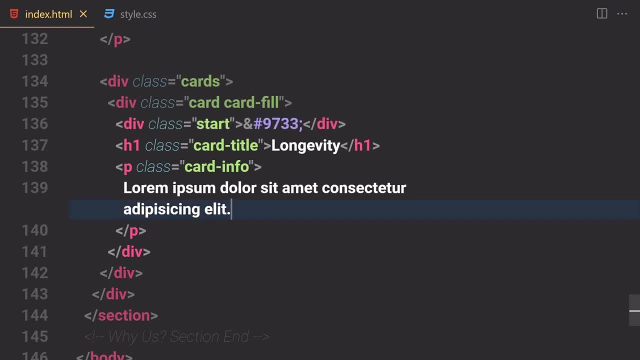 uh, elite would be fine. so, yeah, i guess that would be fine. or we- yeah, i guess that would be fine. or we- yeah, i guess that would be fine. or we can increase the letter, if you want to can increase the letter. if you want to, can increase the letter. if you want to, underneath this paragraph and div, let's. 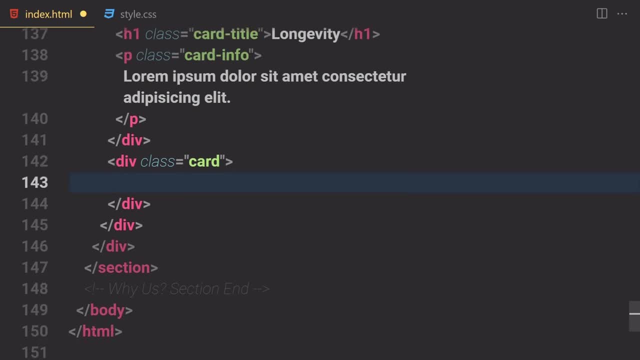 underneath this paragraph and div. let's underneath this paragraph and div. let's just create a new card. just create a new card, just create a new card. so this is going to be a div with the. so this is going to be a div with the. so this is going to be a div with the class of card. then we have h1 with the. 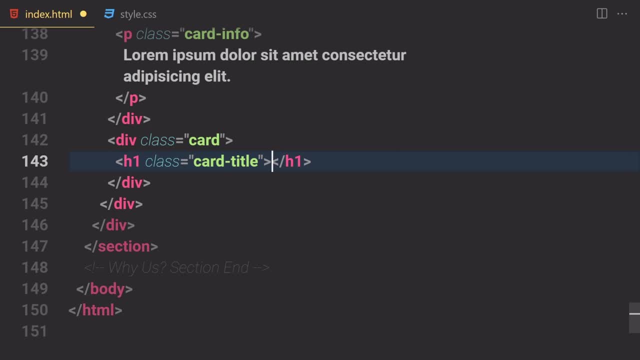 class of card. then we have h1 with the class of card, then we have h1 with the class of card title. let's just put a class of card title. let's just put a class of card title. let's just put a title to it like quantity or quality. 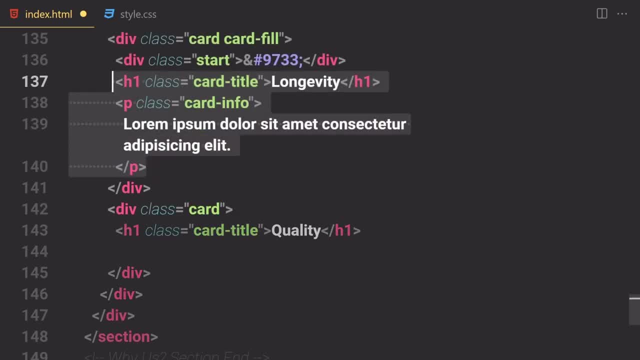 title to it like quantity or quality. title to it like quantity or quality would be fine, and let's just reuse that would be fine, and let's just reuse that would be fine and let's just reuse that paragraph. copy it from here and i'm paragraph. copy it from here and i'm. paragraph, copy it from here and i'm going to paste it right here. so if you going to paste it right here, so if you going to paste it right here, so if you say over there, let's just reuse this, say over there, let's just reuse this, 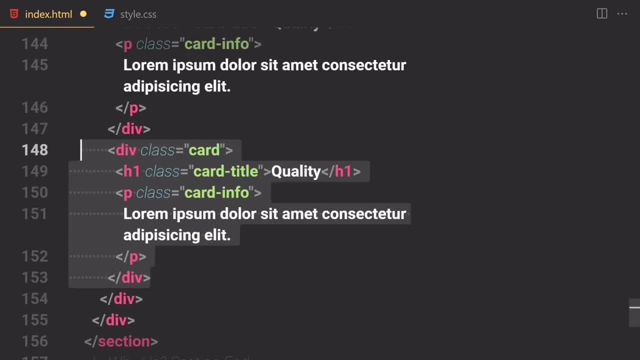 say, over there, let's just reuse this card one more time. so i'm going to just card one more time. so i'm going to just card one more time. so i'm going to just duplicate there. so then we have a card, duplicate there. so then we have a card. 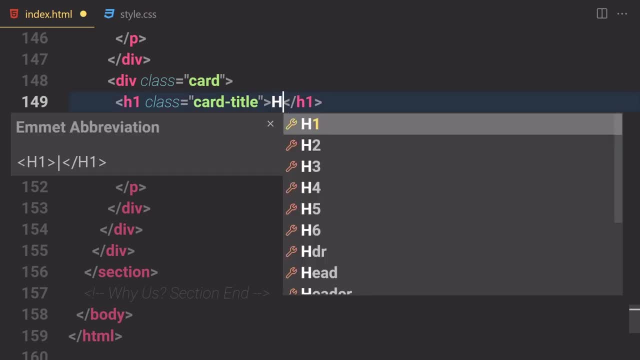 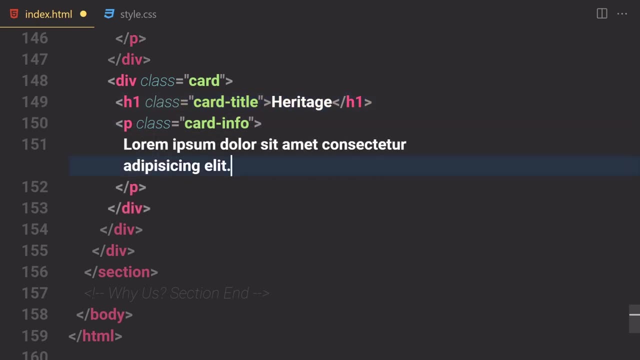 duplicate there. so then we have a card title to be like something else, maybe heritage and heritage, and heritage and the other stuff would be fine the way the other stuff would be fine, the way the other stuff would be fine the way it is. it is now underneath this card. first of all, 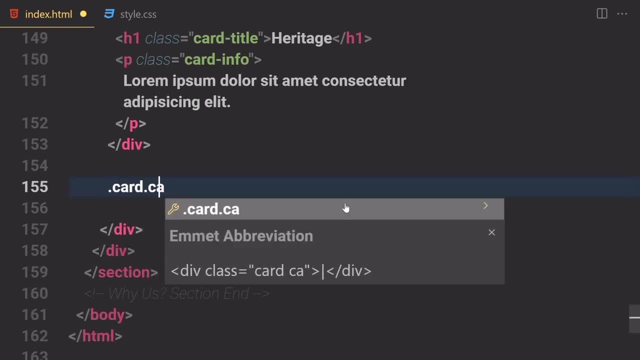 now underneath this card, first of all, now underneath this card. first of all, let's just create a new div with the. let's just create a new div with the. let's just create a new div with the class of car: class of car, class of car and also card. uh fill. and also card uh fill and also card uh fill inside there. what do we have to do, we inside there? what do we have to do, we inside there? what do we have to do? we are going to be writing our star one. are going to be writing our star one. 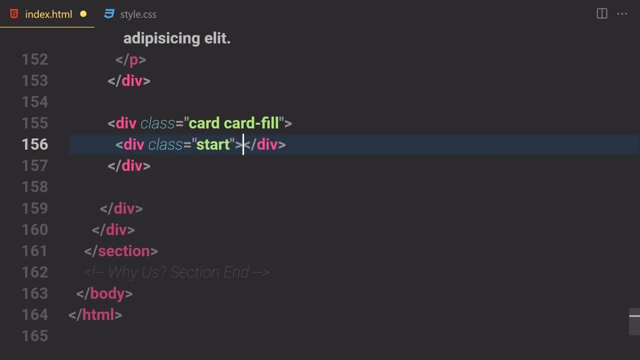 are going to be writing our star one more time. so we have more time, so we have more time, so we have word with a class of star, word with a class of star, word with a class of star. not start, but just a star, did i just? not start, but just a star, did i just? 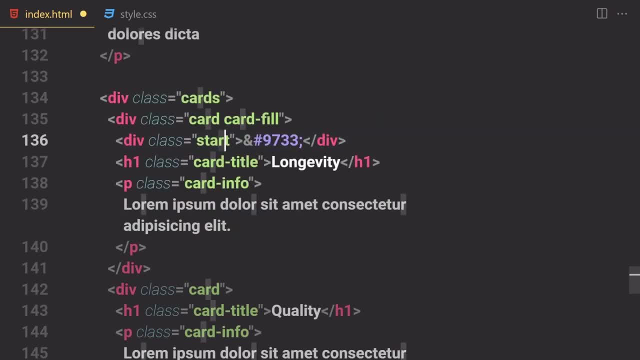 not start, but just a star. did i just spell that start or start? spell that start or start. spell that start or start. it's not a start, it's just a star and it's not a start. it's just a star and it's not a start, it's just a star. and i'm going to also copy that from here. 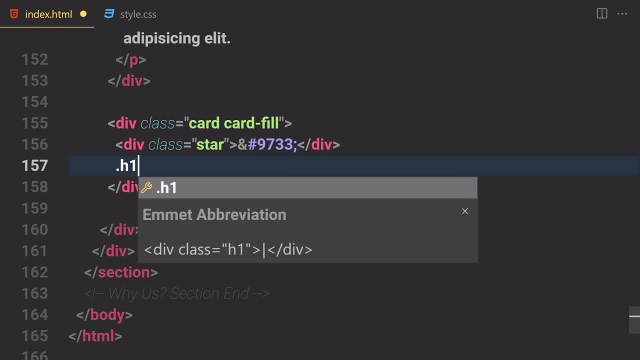 i'm going to also copy that from here. i'm going to also copy that from here and i'm going to be listing right here and i'm going to be listing right here and i'm going to be listing right here. let's just provide each one with the. 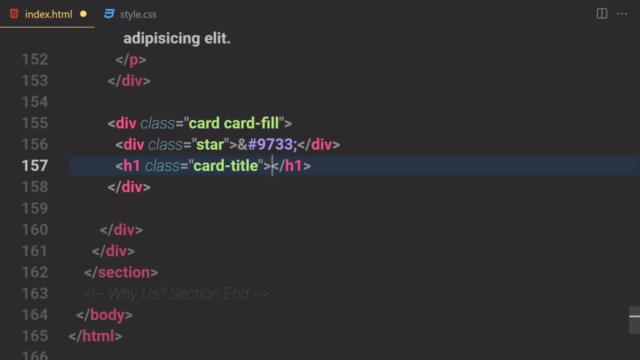 let's just provide each one with the, let's just provide each one with the class of car, class of car, class of car title, and let's just put some title to title and let's just put some title to title and let's just put some title to it like community would be fine. 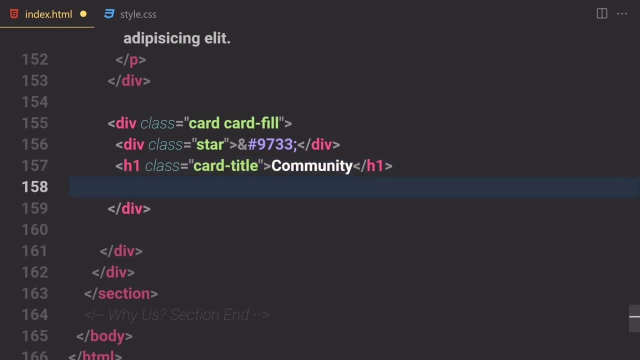 it like community would be fine. it like community would be fine. c-o-w-m-u-n-i-t-y, c-o-w-m-u-n-i-t-y, c-o-w-m-u-n-i-t-y, thanks. so let's just provide a paragraph, thanks. so let's just provide a paragraph. 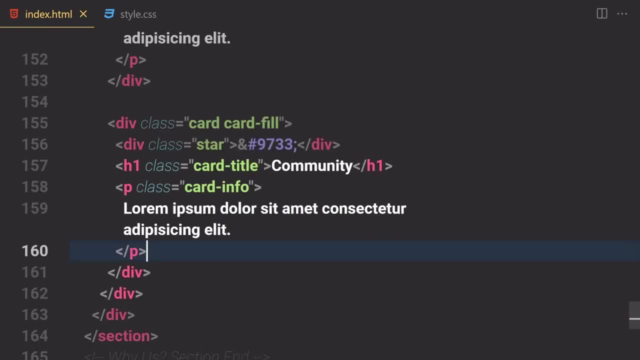 thanks. so let's just provide a paragraph. you know i'm going to copy this. you know i'm going to copy this. you know i'm going to copy this paragraph from there. i'm going to paste paragraph from there. i'm going to paste paragraph from there. i'm going to paste it right here. so if you save a file, we 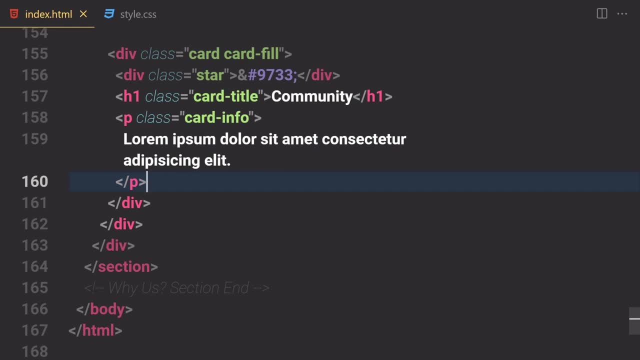 it right here. so if you save a file, we it right here. so if you save a file, we are totally done with this card section, are totally done with this card section, are totally done with this card section. so now let's just get into word style. so now let's just get into word style. 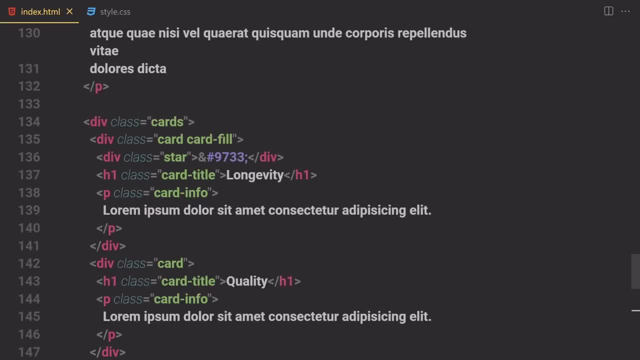 so now let's just get into word style: sheet and knowledge style that i know. sheet and knowledge style that i know. sheet and knowledge style that i know there was a lot of talking, a lot of, there was a lot of talking, a lot of, there was a lot of talking, a lot of typing. so this is air. so if you want to, 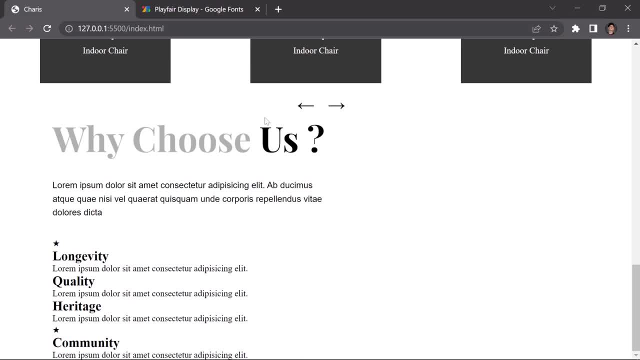 typing, so this is air. so if you want to typing, so this is air. so if you want to check it out, so this is how it looks, check it out. so this is how it looks. check it out. so this is how it looks like for html and this is how it looks. 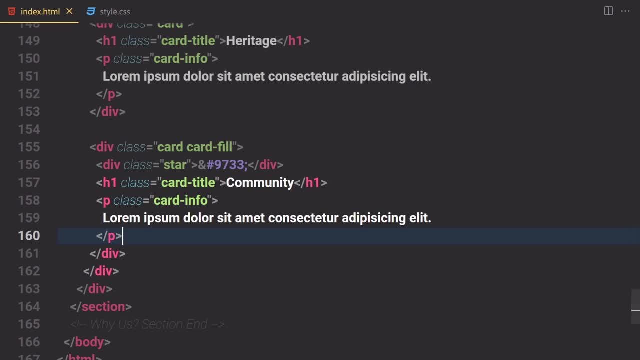 like for html. and this is how it looks like for html. and this is how it looks like like. like in the browser for now. all right, so in the browser for now. all right, so in the browser for now. all right, so now let's jump into our css. and now. now, let's jump into our css. and now, now, let's jump into our css. and now, let's just try a little bit. i'm going to, let's just try a little bit. i'm going to, let's just try a little bit. i'm going to zoom in a bit and let me just write a. 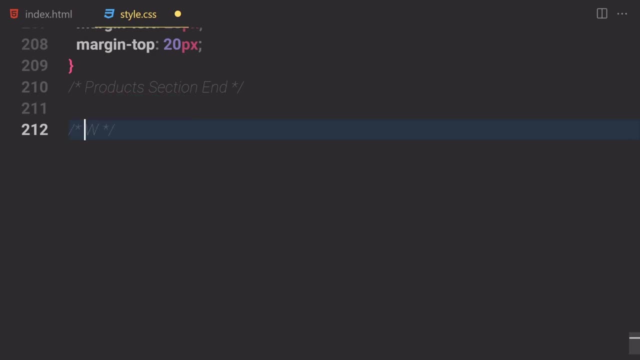 zoom in a bit and let me just write a zoom in a bit and let me just write a comment for myself, like comment for myself, like comment for myself, like uh what, uh what, uh what. why choose? why choose? why choose us question mark section, us question mark section. 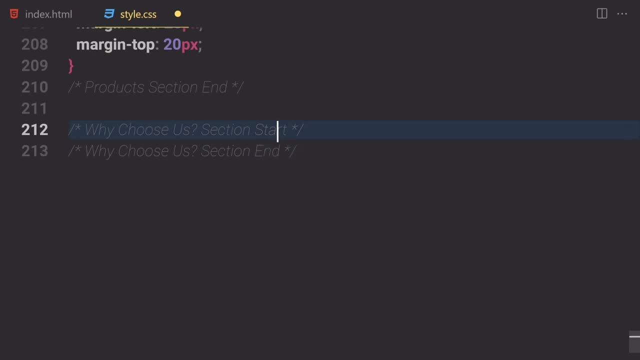 us question mark section: start- okay, so duplicate that. and this start okay, so duplicate that. and this start okay, so duplicate that. and this is going to be the end of that section. so is going to be the end of that section. so is going to be the end of that section. so, inside that we are going to be selecting. 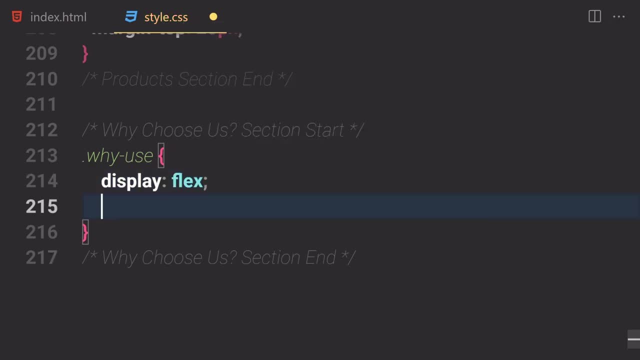 inside that we are going to be selecting, inside that we are going to be selecting, our y us container and display will be our y us container and display will be our y us container and display will be now set to totally flex flex wrap will now set to totally flex flex wrap will. 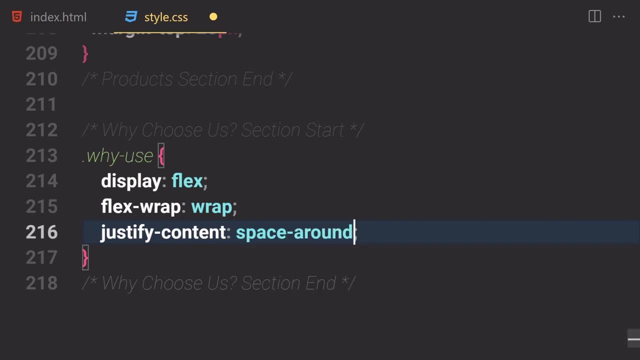 now set to totally flex. flex wrap will be now set to wrapping and justify. be now set to wrapping and justify. be now set to wrapping and justify. counter will be now set to space around. counter will be now set to space around. counter will be now set to space around. align items will be also set to center. align items will be also set to center. align items will be also set to center. margin for the top will be now set to 10. margin for the top will be now set to 10. margin for the top will be now set to 10 rems. 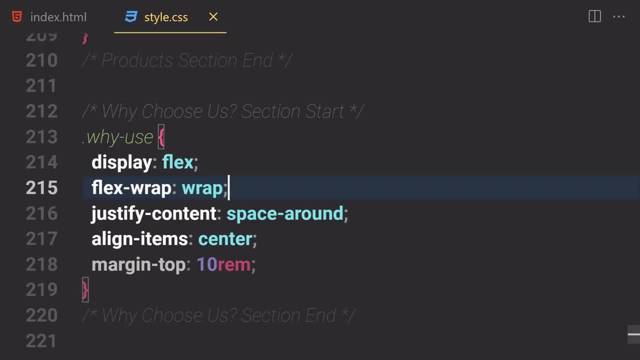 rems, rems. and now if you sell a file and nothing is? and now if you sell a file and nothing is? and now if you sell a file and nothing is working the way we expect them to work, working the way we expect them to work, working the way we expect them to work? let's just see. 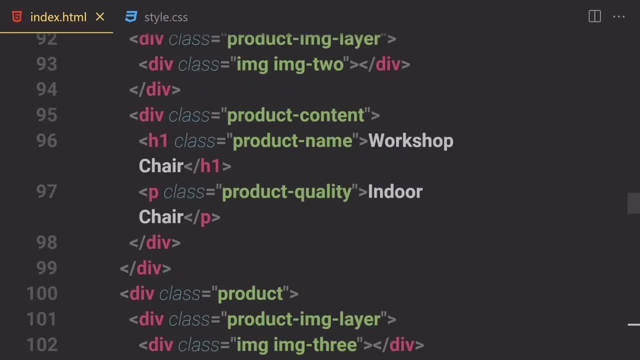 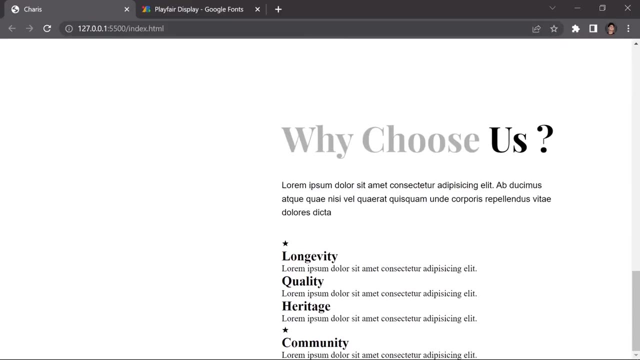 let's just see. let's just see: something is wrong, so we have popularity. something is wrong, so we have popularity. something is wrong, so we have popularity. product, product, product. and then we have our container watch. oh, and then we have our container watch. oh, and then we have our container watch. oh, my goodness, not why use, but just why us. 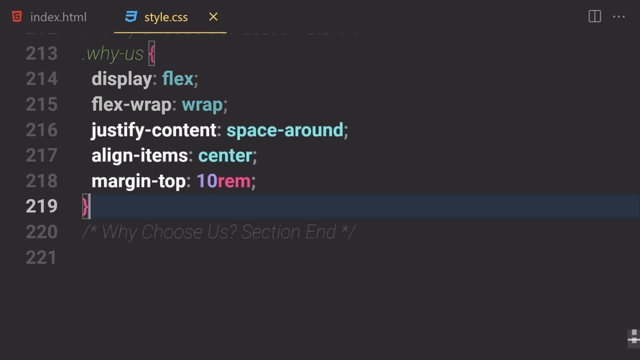 my goodness, not why use, but just why us. my goodness, not why use, but just why us. and this is how it looks like for now. and this is how it looks like for now. and this is how it looks like for now. my bad, sorry, and now let's just start. 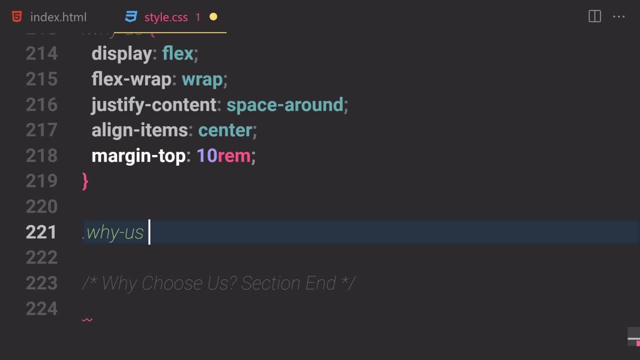 my bad, sorry, and now let's just start. my bad sorry, and now let's just start working on our image layer. so why us in working on our image layer? so why us in working on our image layer? so why us in this case not? why use this case not? why use? 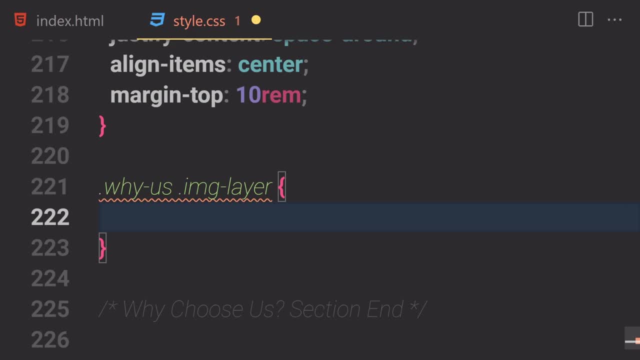 this case not. why use don't be stupid like me. and then image don't be stupid like me. and then image don't be stupid like me. and then image layer, layer, layer, and with i'm going to give like 400 and with i'm going to give like 400. 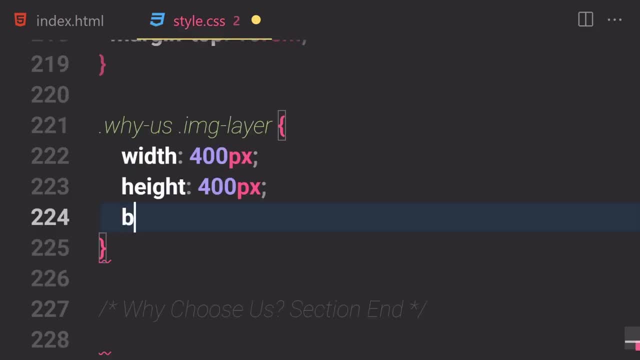 and with i'm going to give like 400 pixel pixel pixel and height will be also 100 400 pixel and height will be also 100 400 pixel and height will be also 100 400 pixel. background color will be now set to like: 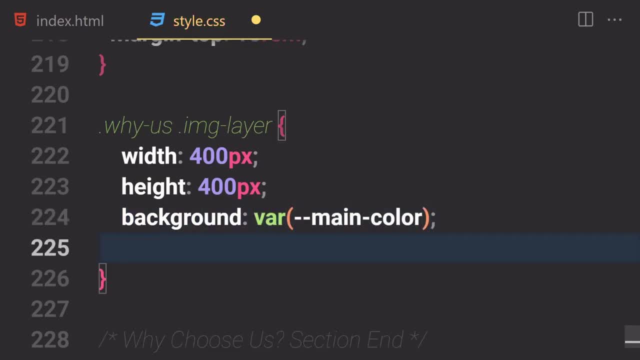 background color will be now set to like. background color will be now set to like: main color: c o l o r- main color. c o l o r. main color. c o l o r and border radius: i'm going to give like. and border radius: i'm going to give like. 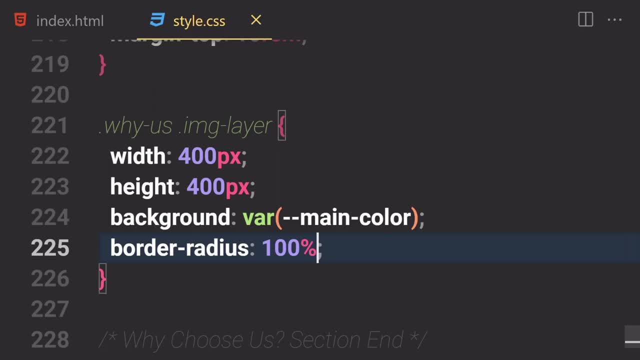 and border radius. i'm going to give like 100 and if you sell that, and this is how 100, and if you sell that, and this is how 100, and if you sell that, and this is how it looks like. i'm going to zoom out and 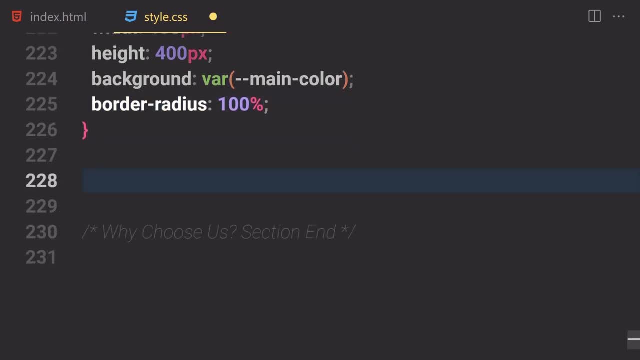 it looks like i'm going to zoom out. and it looks like i'm going to zoom out and now let's just take care of that image. now, let's just take care of that image. now let's just take care of that image layer and that image inside that layer. 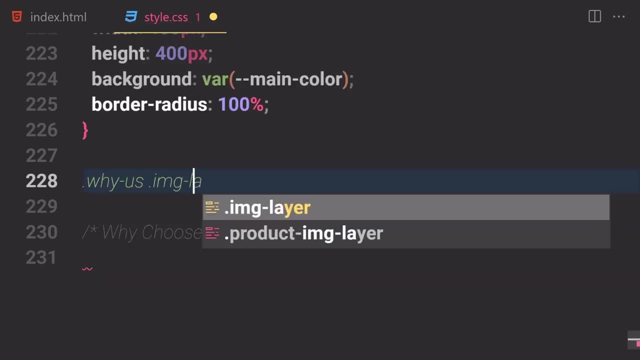 layer and that image inside that layer layer and that image inside that layer. so i'm going to write a y? us, then image. so i'm going to write a y us, then image. so i'm going to write a y us, then image layer and then img class. 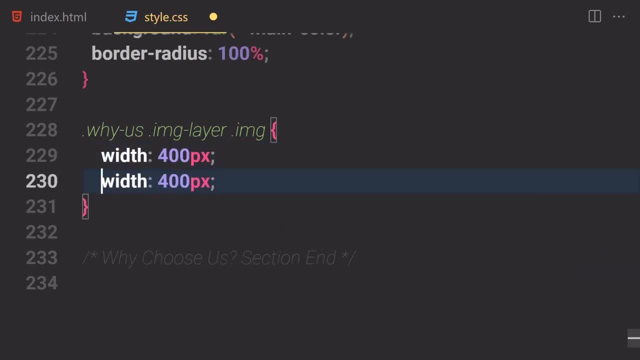 layer and then img class layer and then img class. so i'm going to provide a width of like. so i'm going to provide a width of like. so i'm going to provide a width of like 400 pixel, and the height will be also 400 pixel and the height will be also. 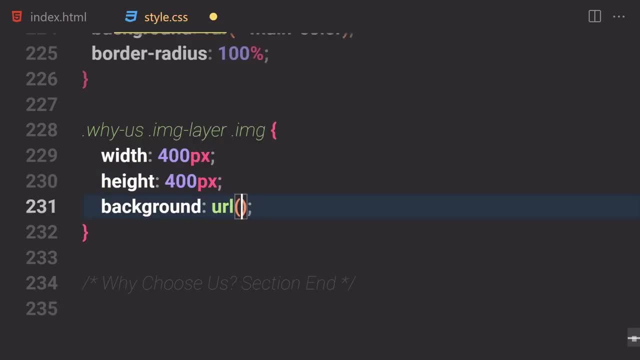 400 pixel and the height will be also 400 pixel. background color, not color, but 400 pixel. background color, not color, but 400 pixel. background color, not color, but a background image will be url. go to the. a background image will be url. go to the. 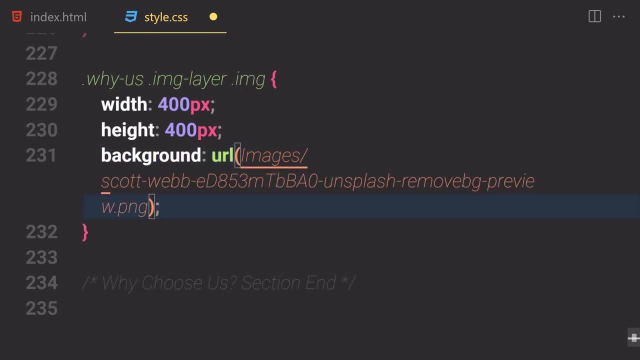 a background image will be url. go to the images and check out that one. so i'm images and check out that one. so i'm images and check out that one. so i'm going to just select that one. going to just select that one, going to just select that one. let's just provide a background size of 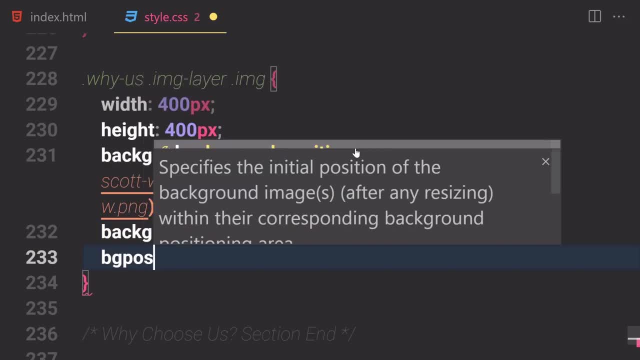 let's just provide a background size of. let's just provide a background size of totally cover and the background position totally cover and the background position totally cover, and the background position will be now set to totally center. okay, so will be now set to totally center, okay, so, will be now set to totally center. okay, so, if you save that and this is how it, if you save that, and this is how it, if you save that, and this is how it looks like right now- okay, so now let's looks like right now. okay, so now let's. 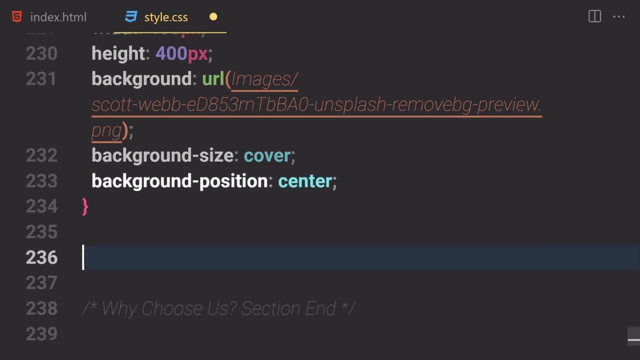 looks like right now. okay, so now let's just take care of this area like cards. just take care of this area like cards, just take care of this area like cards and stuff. so first of all, let's just and stuff. so, first of all, let's just. 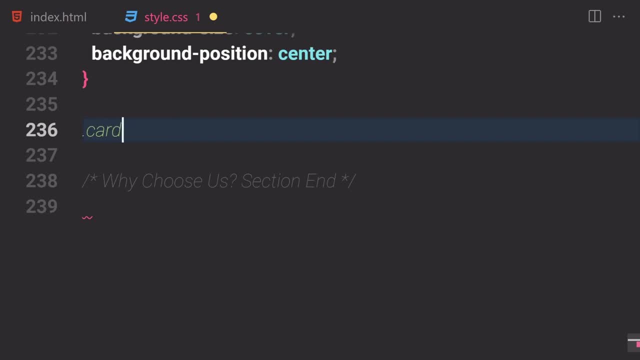 and stuff. so, first of all, let's just select or cards- not buttons card, but select. or cards, not buttons card, but select. or cards, not buttons card, but just a card is, just a card is, just a card is, and let's just provide a display of grid. 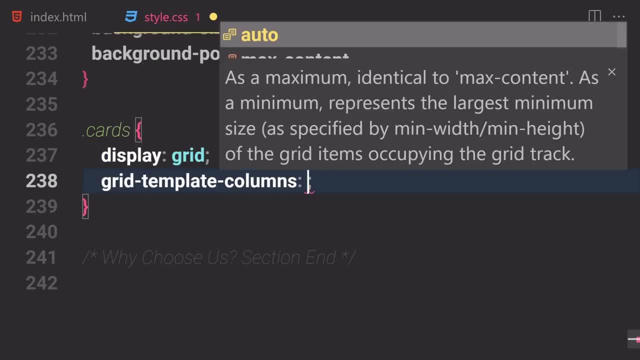 and let's just provide a display of grid. and let's just provide a display of grid on it. and grid template: uh columns, so we on it. and grid template: uh columns, so we on it. and grid template, uh columns. so we want two columns of 2fr and 2fr. so if 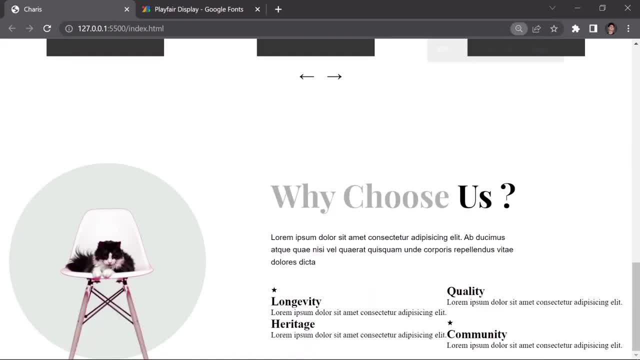 want two columns of 2fr and 2fr. so if want two columns of 2fr and 2fr, so if you sell that, you sell that. you sell that. uh okay, uh okay, uh okay. and this is how it looks like right now. and this is how it looks like right now. 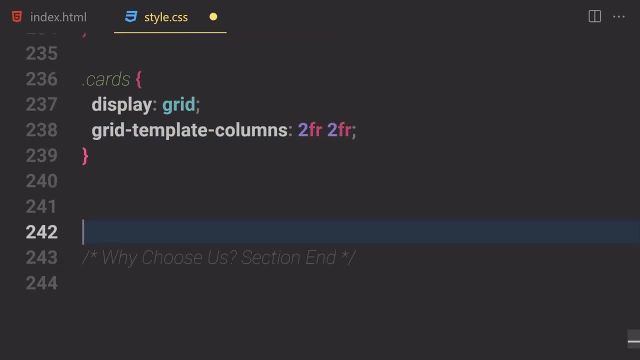 and this is how it looks like right now. so now, let's just take care of this each. so now, let's just take care of this each. so now, let's just take care of this: each card inside that card section. so i'm card inside that card section, so i'm. 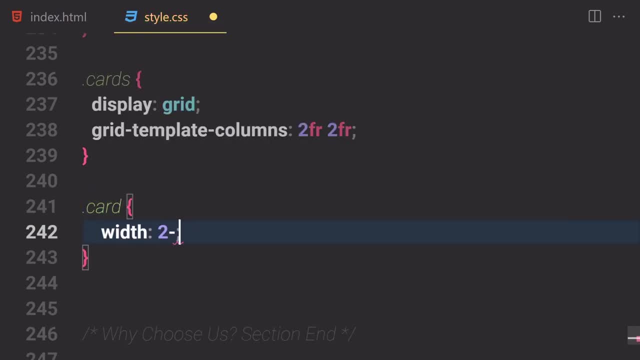 card inside that card section. so i'm gonna just write like a card, gonna just write like a card, gonna just write like a card and let's just provide a width of like 200, and let's just provide a width of like 200, and let's just provide a width of like 200 pixel and height will be 150 pixel. 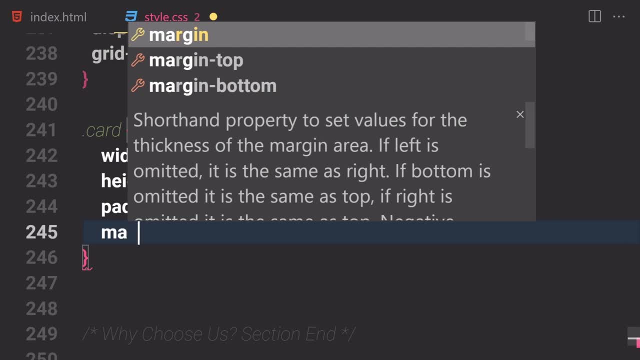 pixel and height will be 150 pixel. pixel and height will be 150 pixel padding. i'm going to give him like 20 padding. i'm going to give him like 20 padding. i'm going to give him like 20 pixel all around and margin. pixel all around and margin pixel all around and margin for the top. i'm going to give him like for the top. i'm going to give him like for the top. i'm going to give him like: 40 pixel, let's just provide a border. 40 pixel, let's just provide a border. 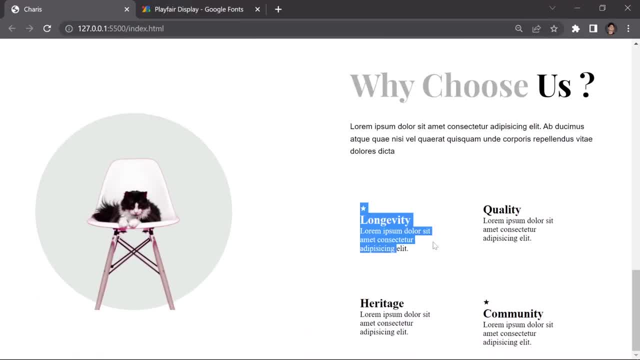 40 pixel. let's just provide a border radius of five pixels. if you save that radius of five pixels, if you save that radius of five pixels, if you save that, and this is how each of the card looks, and this is how each of the card looks. 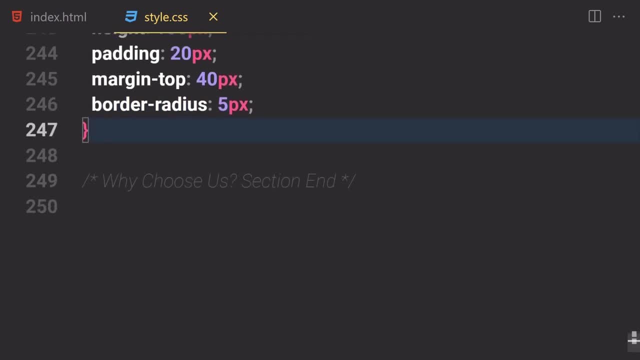 and this is how each of the card looks like right now: okay, like right now. okay, like right now, okay. so what do we have to do? we are going to. so what do we have to do? we are going to. so what do we have to do? we are going to be using that card fill. 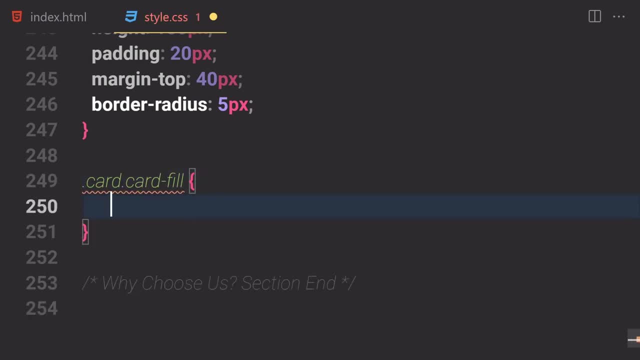 be using that card, fill, be using that card, fill and let's just use card and then card, and let's just use card and then card and let's just use card and then card and fill if the card is filled, so we, and fill if the card is filled, so we. 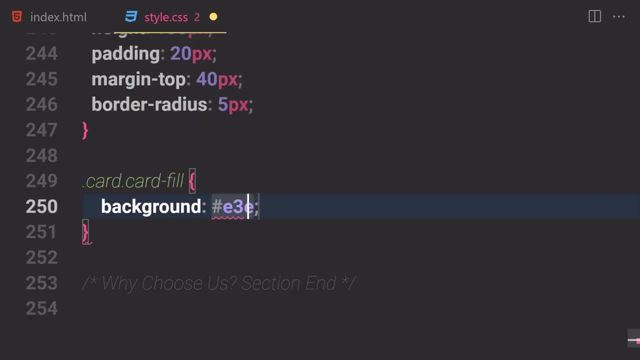 and fill if the card is filled. so we want to change the color of that to be, want to change the color of that to be, want to change the color of that to be like: uh, i don't know e3 e. like: uh, i don't know, e3 e. 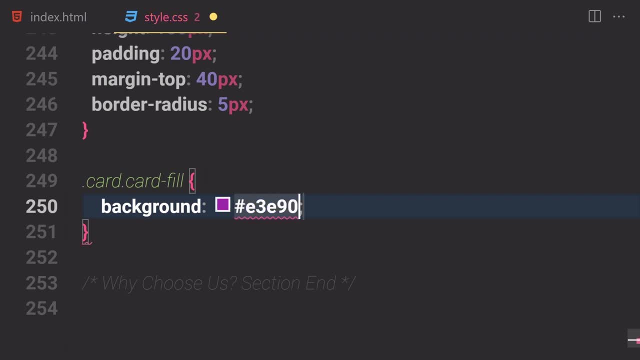 like uh, i don't know, e3, e, uh, not three again, but just add kind of uh, not three again, but just add kind of uh, not three again, but just add kind of a long color. so and oh my god, uh, e4, 90. i mean, so this is going to be the. 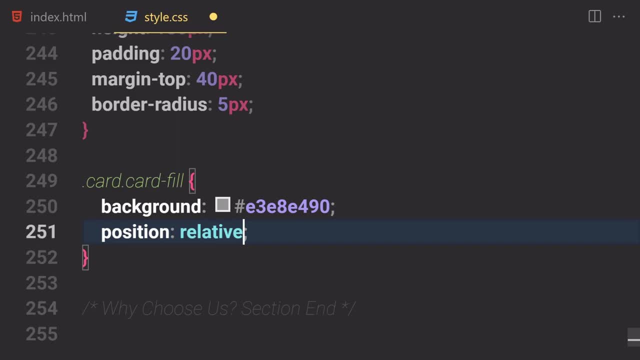 90. i mean so this is going to be the 90. i mean so this is going to be the card color, and position will be now set card color and position will be now set card color and position will be now set to to to relative. so if you save that, so here you. 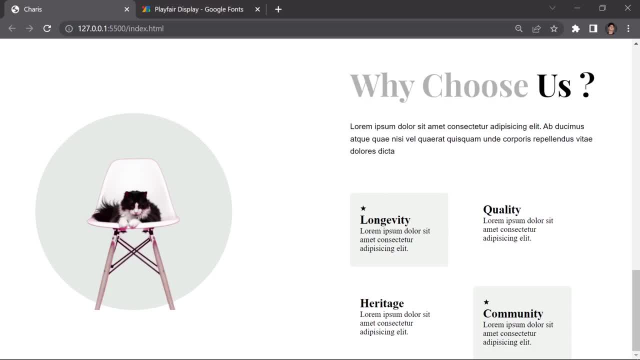 relative. so if you save that, so here you relative. so if you save that, so here you can see, both of them will have the class. can see both of them will have the class. can see both of them will have the class of card fill. so that's why we are now. 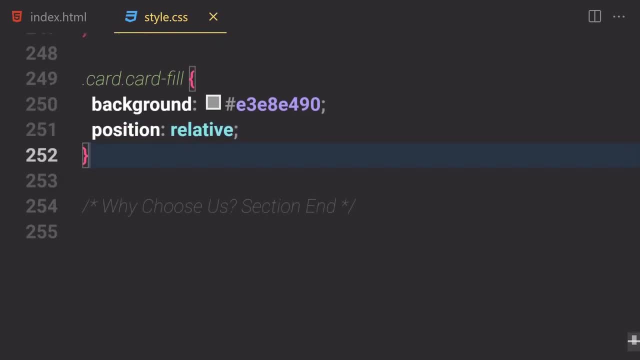 of card fill. so that's why we are now of card fill, so that's why we are now getting that color anyways. so now let's getting that color anyways. so now let's getting that color anyways. so now let's just take care of that card. just take care of that card. 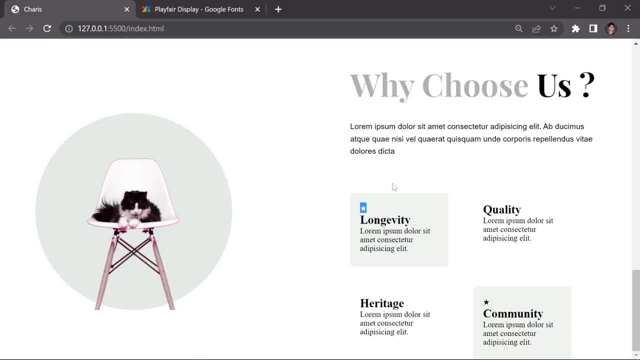 just take care of that card uh fill, and then that star which we uh fill, and then that star which we uh fill, and then that star which we provide right here. so i'm gonna just provide right here, so i'm gonna just provide right here, so i'm gonna just write like card and then card. 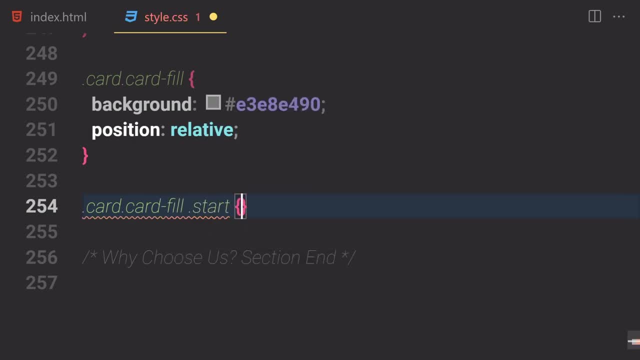 write like card and then card. write like card and then card. if that card is filled, so we want to. if that card is filled, so we want to. if that card is filled, so we want to. select that star, select that star, select that star, okay. so we want to provide a width of. 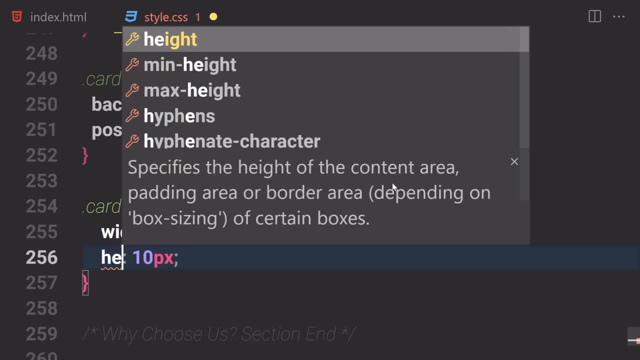 okay, so we want to provide a width of: okay, so we want to provide a width of like 100, not 100, but 10 pixel, and the like 100, not 100, but 10 pixel, and the like 100, not 100, but 10 pixel, and the height will be also 100, not 100 pixel. 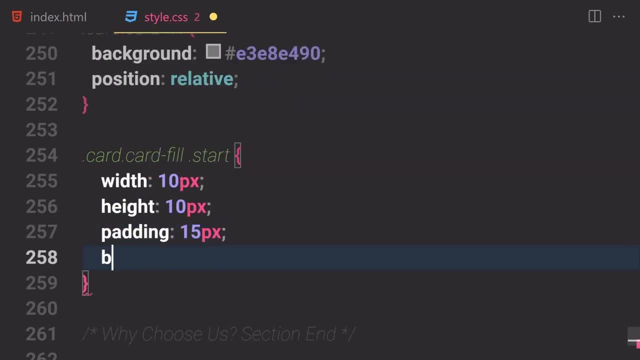 height will be also 100, not 100 pixel. height will be also 100- not 100 pixel, but 10 pixel, and padding will be 15 but 10 pixel and padding will be 15 but 10 pixel and padding will be 15 pixel and border radius will be 100. 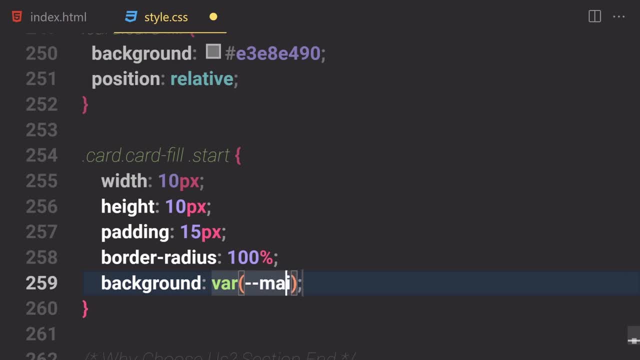 pixel and border radius will be 100 pixel and border radius will be 100, and let's just use the background color and let's just use the background color and let's just use the background color of that same background, of like primary, of that same background of like primary. 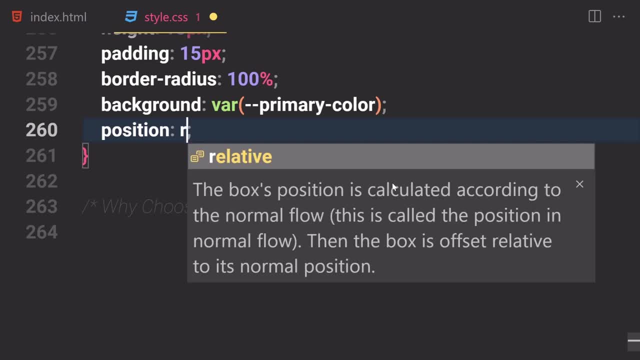 of that same background, of, like, primary color. okay, so color, okay, so color, okay, so let's just use the position of absolute. let's just use the position of absolute. let's just use the position of absolute. the other one was relative, so this one. the other one was relative, so this one. 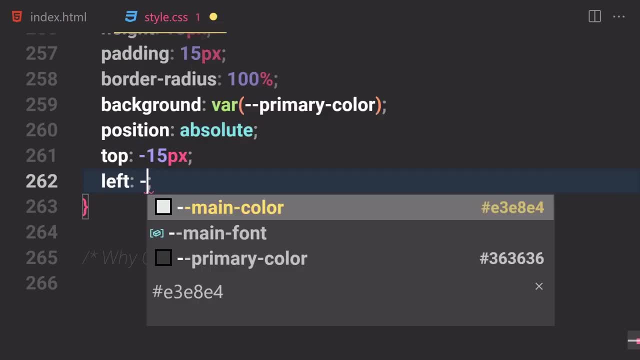 the other one was relative, so this one will be now absolute. so 15 pixel for the will be now absolute. so 15 pixel for the will be now absolute. so 15 pixel for the top for the left. we want negative 10. top for the left: we want negative 10. 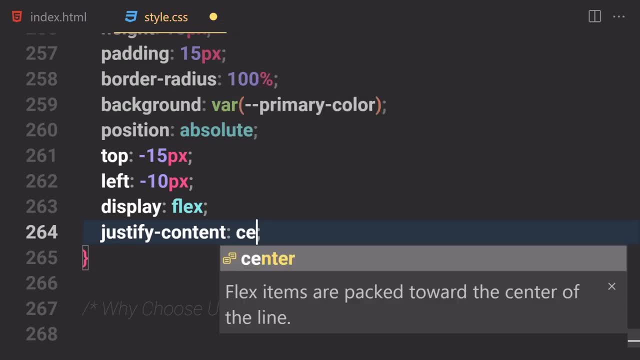 top. for the left. we want negative 10 pixels, so display will be now totally pixels. so display will be now totally pixels. so display will be now totally centered. justify counter will be center centered. justify counter will be center centered. justify counter will be center. uh, align items will be now center and. 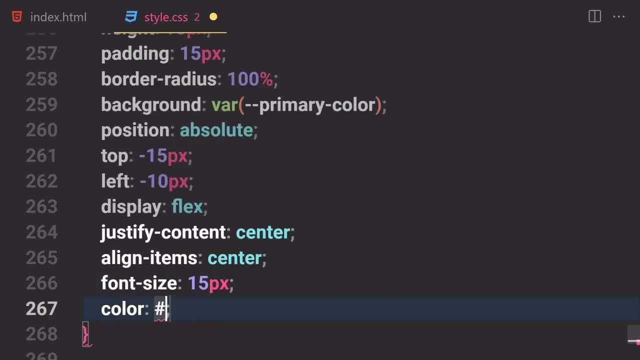 uh align items will be now center and uh align items will be now center and font size. let's just increase that to 15 font size. let's just increase that to 15 font size. let's just increase that to 15 pixel and color will be totally white. 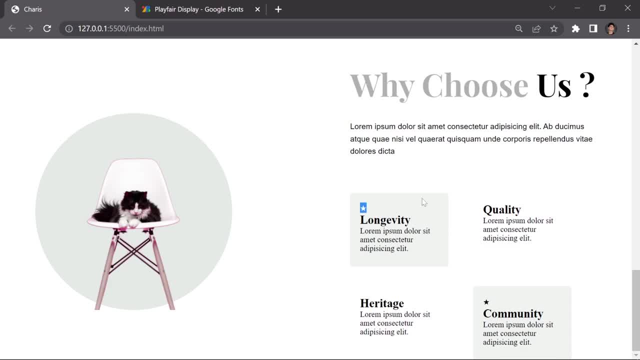 pixel and color will be totally white. pixel and color will be totally white. okay, so if you sell a file, and let's okay. so if you sell a file, and let's okay. so if you sell a file, and let's just see what's going on, so we have a 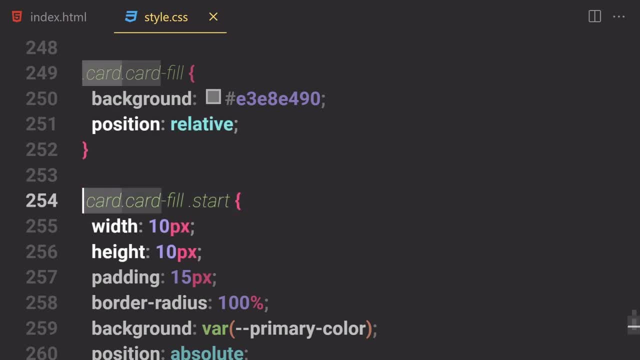 just see what's going on. so we have a. just see what's going on. so we have a card, card, card. then we have a card fill, so let's just then we have a card fill, so let's just then. we have a card fill, so let's just remove this card from here. so if you 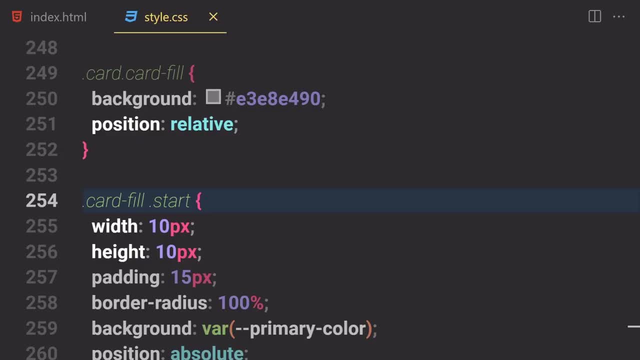 remove this card from here. so if you remove this card from here, so if you sell that, sell that, sell that, okay, something is not working. okay, something is not working. okay, something is not working. this is not a start. man start so seven. this is not a start. man start so seven. 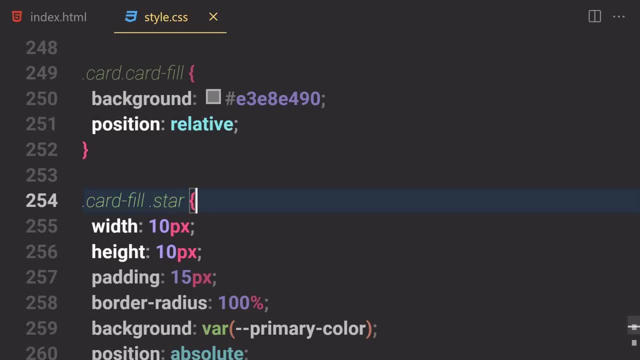 this is not a start man, start. so seven. and now here you can see why am i. and now, here you can see why am i. and now, here you can see why am i getting. why am i writing start, it's it's getting. why am i writing start, it's it's. getting. why am i writing? start it's. it's just a star, all right. so now here you. just a star, all right. so now here you. just a star, all right. so now here you can see it's working the way we expect. can see it's working the way we expect. 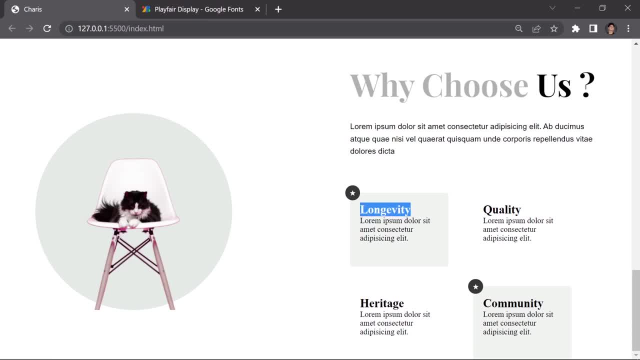 can see it's working the way we expect them to work, them to work, them to work. now, let's just take care of these. um what now? let's just take care of these? um what now? let's just take care of these. um what do we call it? the h1? so let's just 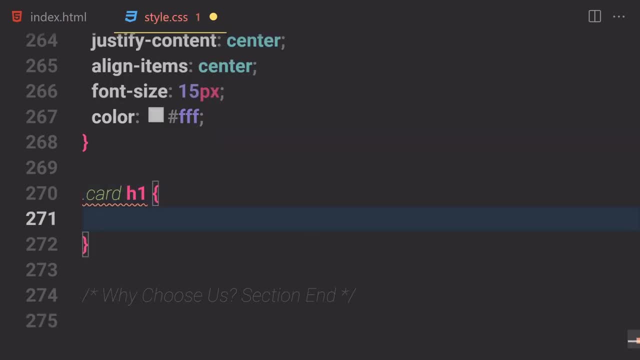 do we call it the h1? so let's just do we call it the h1. so let's just write write, write uh card and h1. so we are going to be write uh card and h1. so we are going to be write uh card and h1. so we are going to be changing the color to be totally black. 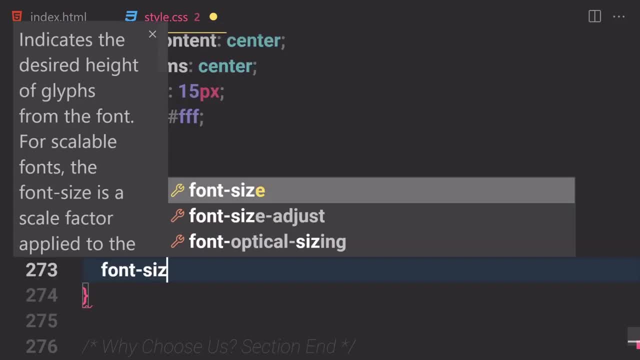 changing the color to be totally black. changing the color to be totally black and the font family will be now set to: and the font family will be now set to. and the font family will be now set to: sans serif: sans serif, sans serif. the font size: i'm going to increase that. 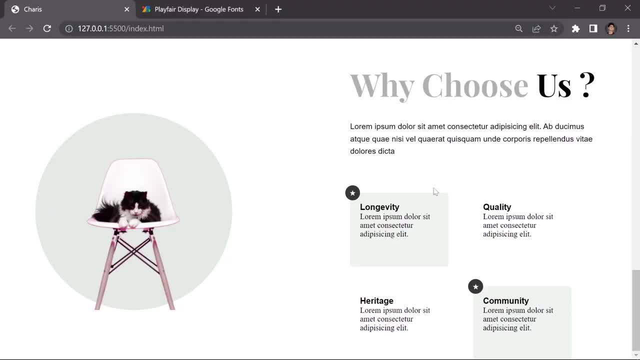 the font size. i'm going to increase that the font size. i'm going to increase that to like 70 pixel. so if you sell that to like 70 pixel, so if you sell that to like 70 pixel, so if you sell that, and this is how it looks like right now, 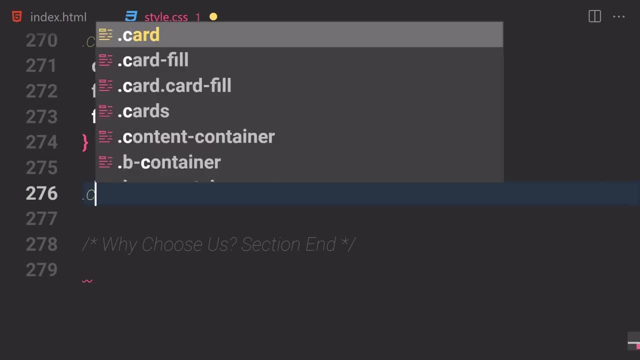 and this is how it looks like right now. and this is how it looks like right now. so now let's just take care of that. so now let's just take care of that paragraph as well. so we are going to be writing a card and then selecting that paragraph, and let's 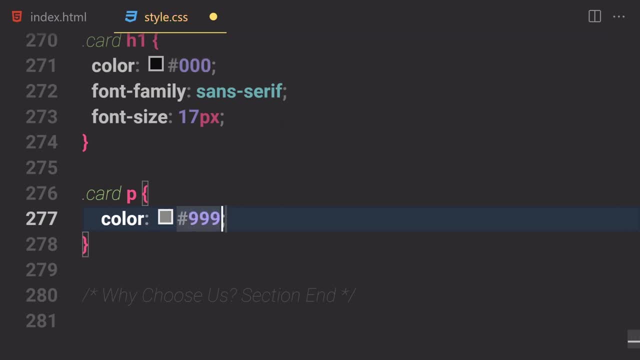 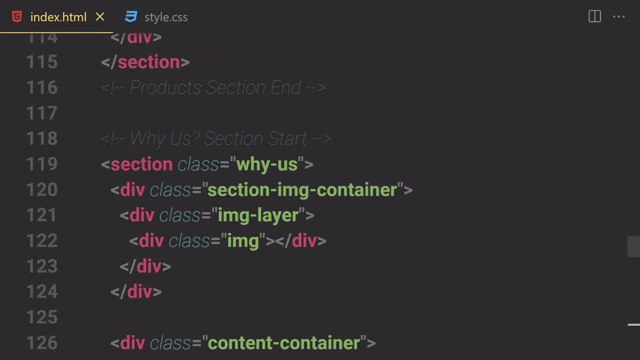 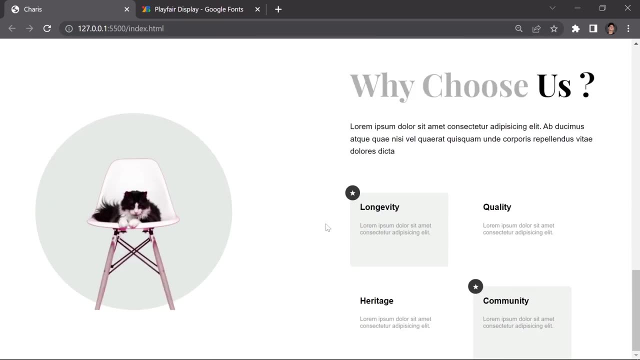 now, okay. so if you want to put a lot of text in there, so you can, or you know what i'm going to, just leave it the way it is. so if you want to provide a lot of color- and not a lot of colors, but a lot of text- so you can also provide that anyway. so that was the end of why choose a section. 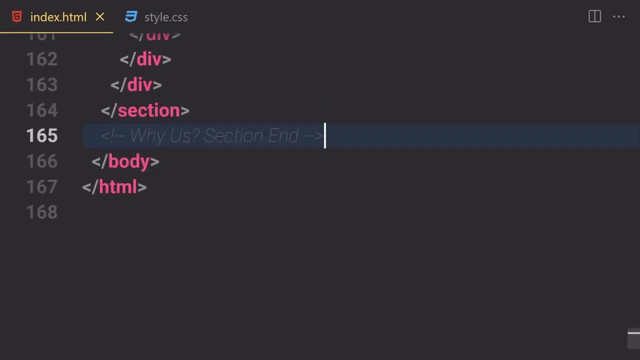 so i'm going to just go to the bottom right here and now let's just take care of that features section. so features section start, duplicate that, and then this is going to be the end of that feature section. so now let's just write a section with the class of features and now inside 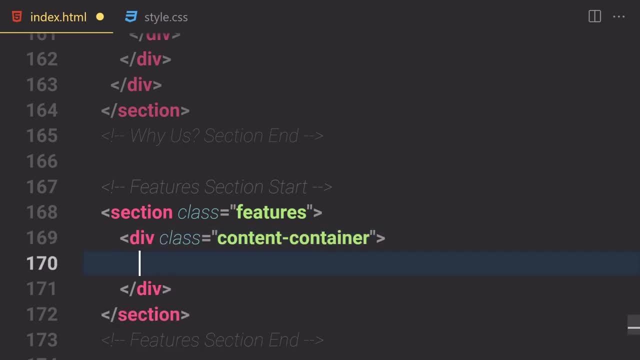 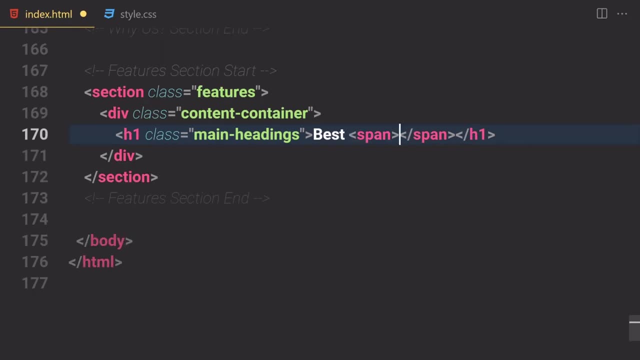 there we are going to be creating a div with the class of colors content container. okay, so let's just write h1 with the class of main headings. best span it to. let's just zoom out features. okay, so if you save that, this is how it looks like. 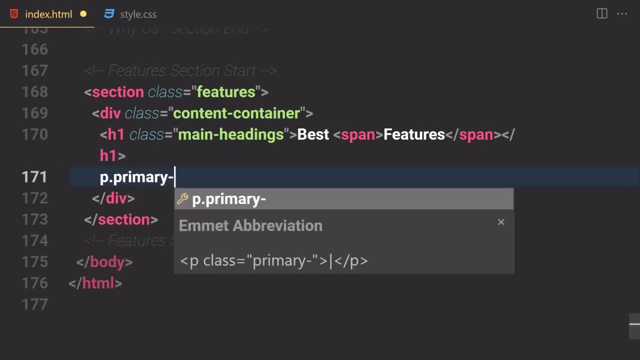 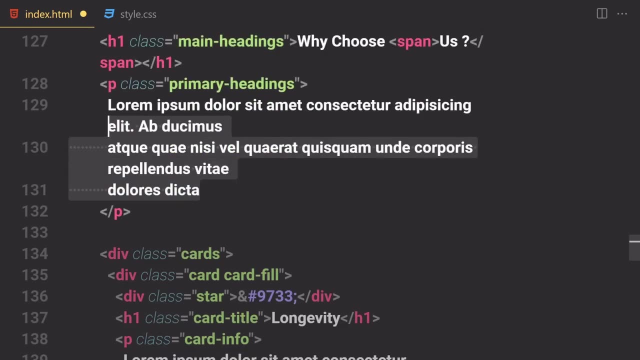 underneath this h1, we're going to be writing paragraph with the class of primary heading, or headings to be precise, and i'm going to be just getting that primary kind of a heading from here, copy that and come to the bottom and i'm going to paste it right here inside this paragraph. 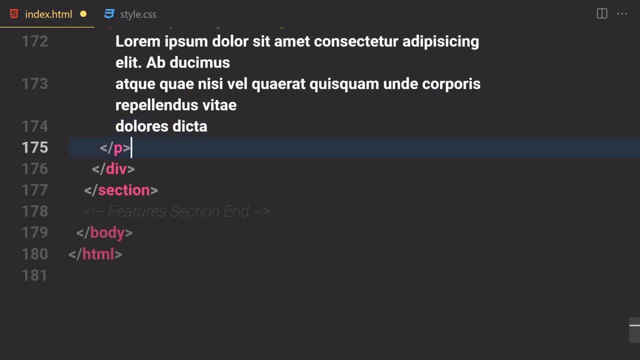 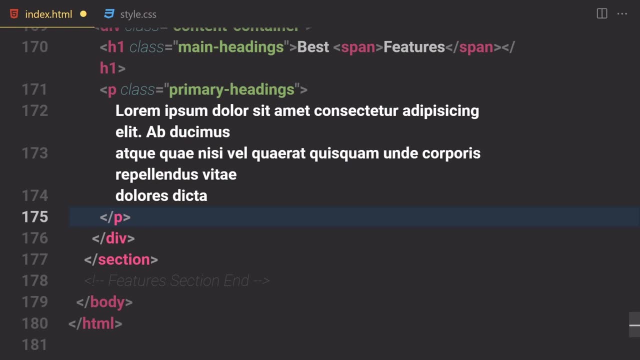 and now we're going to be creating a div and i'm going to paste it right here inside this paragraph. what else do we have to do now? let's just create that cards one more time. so what can i do? you know, underneath this paragraph, i'm going to be writing a card. 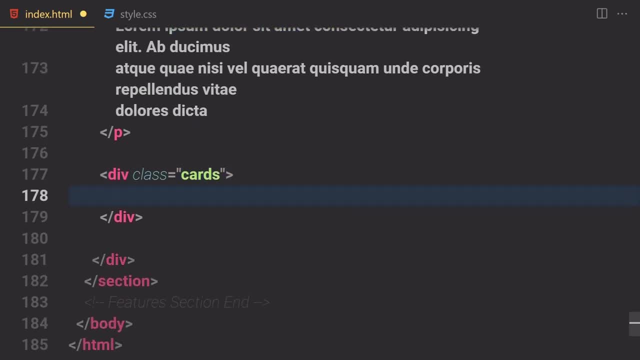 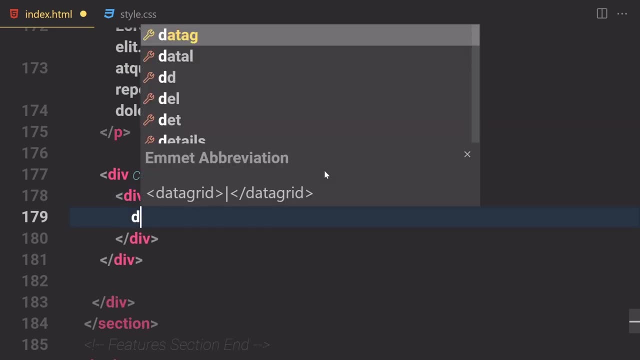 uh yeah, div of the class: class of cards. inside there we are going to be placing over different kind of cards. so we have a card and then card fill. so this one is going to be the card of fill, and now let's just write a div with the class of star. so we are going to be also reusing that star. 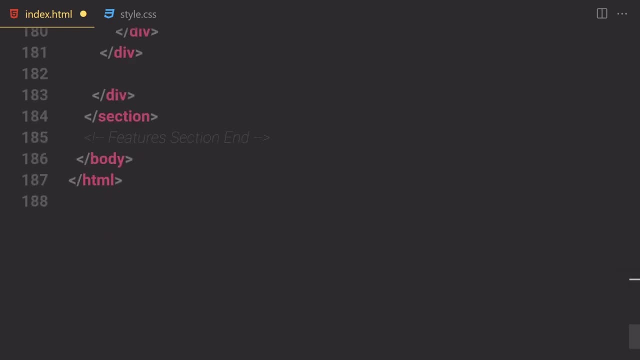 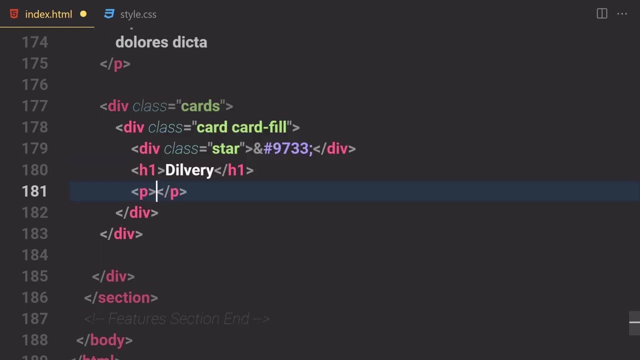 i'm going to copy that from here. it's kind of a lot of uh symbols, right, so i'm going to just place it right here and let's just write h1 of delivery. let's just use that paragraph one more time. i'm going to copy all of their text. i'm going to paste it right here. oh, you know what uh, their? 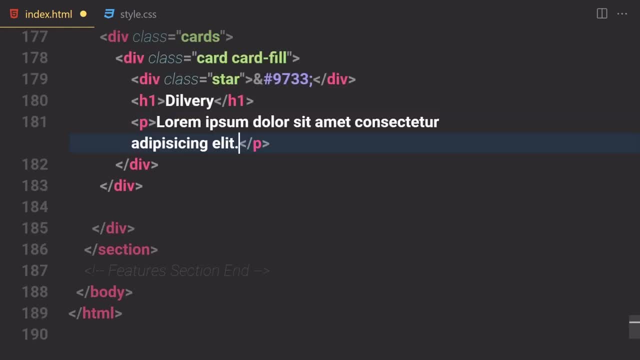 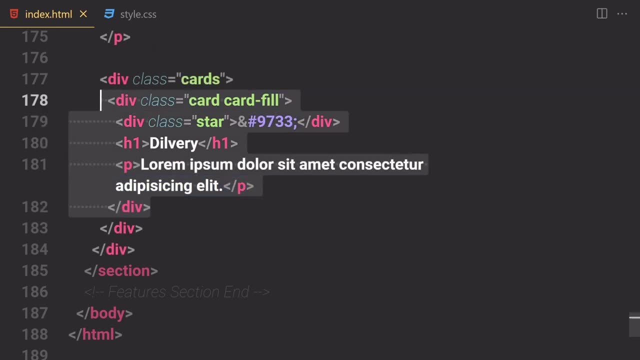 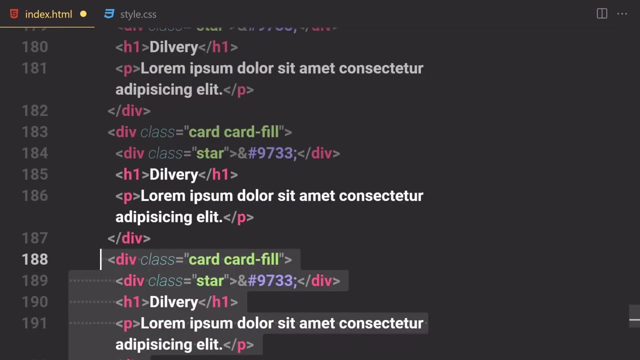 text would be fine. so i'm going to copy that from there and i'm going to paste it right here. okay, so this is going to be the card fill and let's just duplicate that a few times. so i'm going to just duplicate that one time and two times. so let's just change these titles to be like something else. 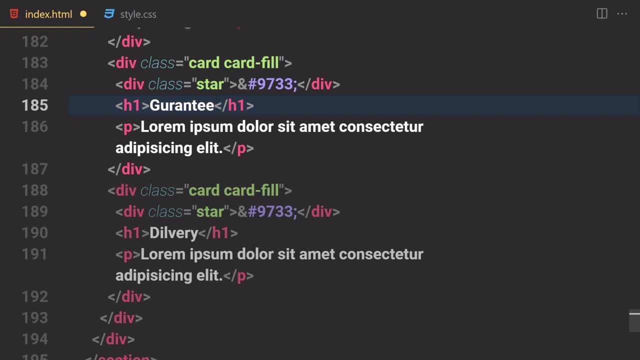 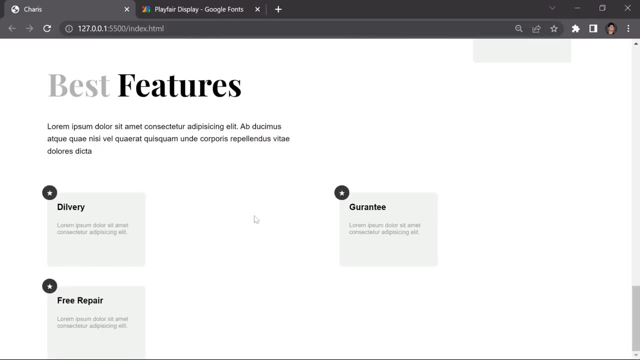 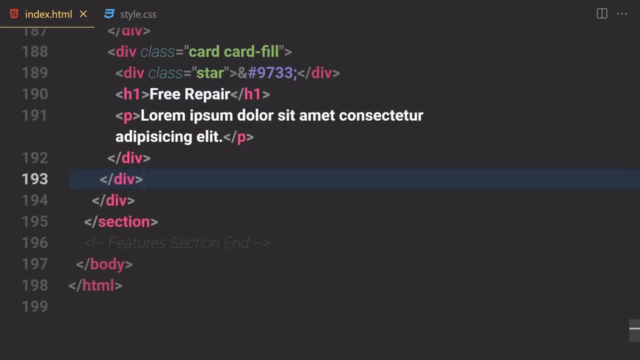 guarantee and then free repair, re repair, like so. so if you sell that- and this is how it looks like for now, i know it's looking awful, so now let's just take care of the area. but before we do, we have to also write an image container as well underneath all of these divs. now let's just go. 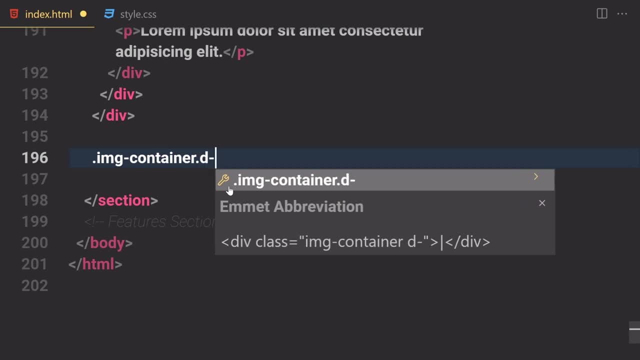 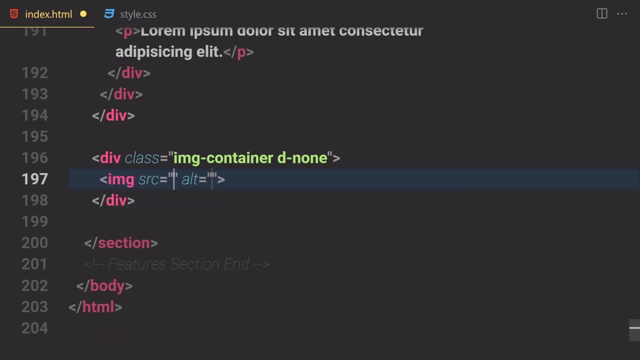 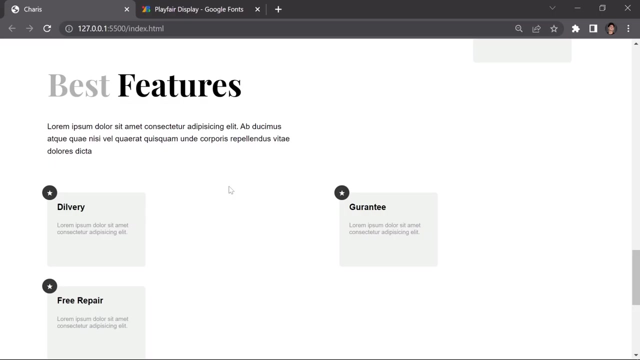 right there with the class of img and container and also display will be none so non. so once we hit some sort of a certain media query, so we want to remove that. so now let's just get that image and which is that bruno or whatever you want to call that. so if you save that, and this is how it, 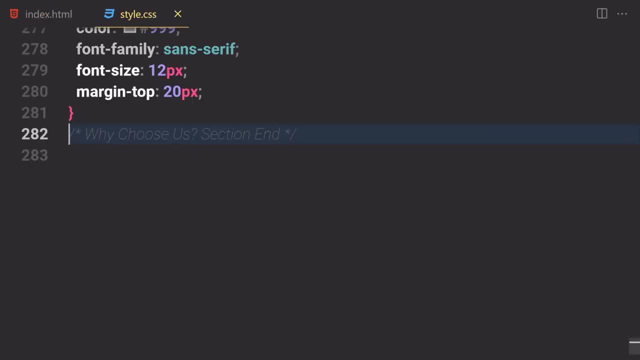 looks like right now. okay, so now let's just get into our css. and now let's just style that a bit. i'm going to write a comment for myself, like: features section start, duplicate, then feature section end. and now inside that let's just select our features section. i'm going to give a margin. 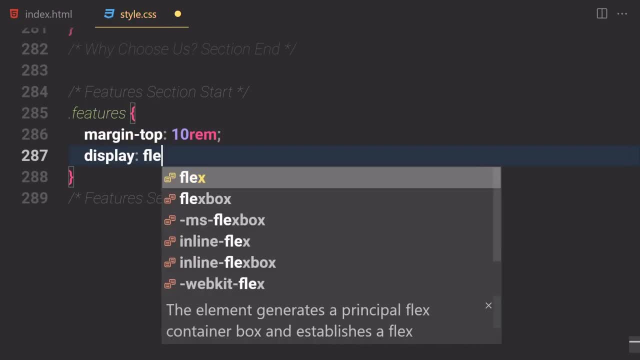 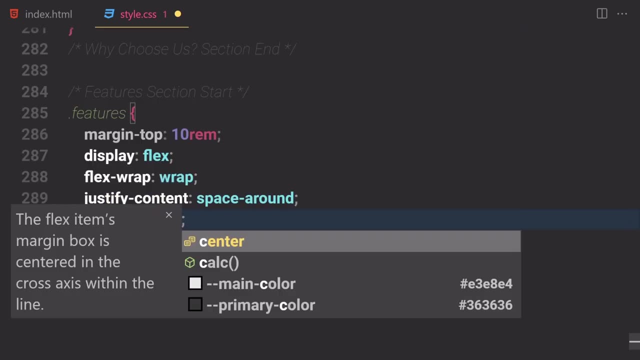 for the top, like 10 ram and display will be totally flex. uh, flex ram will be now set to wrap and justify. content will be now set to space around. align items will be now set to totally center, and now let's just start working. or you know, let me just save that and this is how currently. 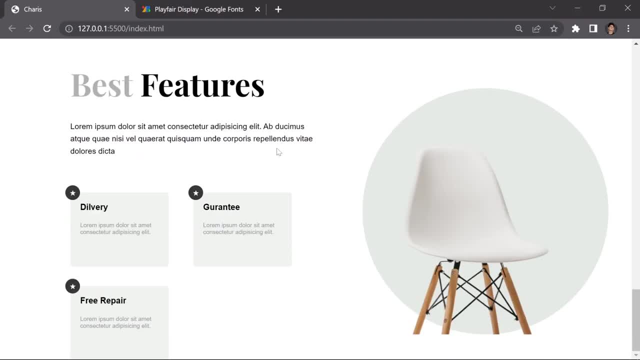 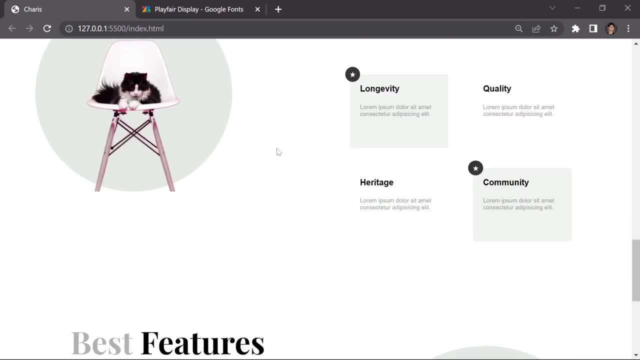 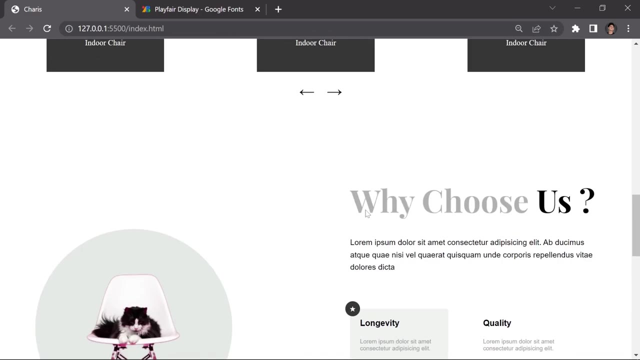 things looks like and i guess this looking awesome. i don't have for a lot of uh, other things, so i guess that's looking awesome. you know, i don't have to do anything else for this feature section, or we can decrease the size of the images if you want to, but i guess that's looking cool. 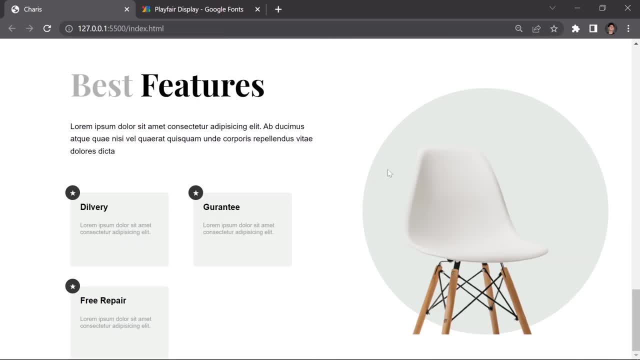 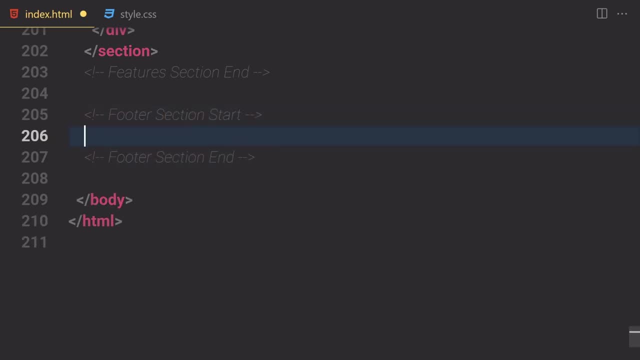 so finally, let's just take care of the forward section. all right, so now let's just start working on our folder section. start duplicate. then for section n: okay, so let me just write a folder. inside this folder we are going to be writing a div with the class of logo container inside there. 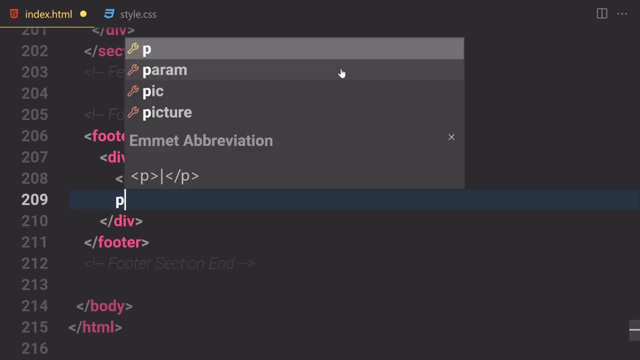 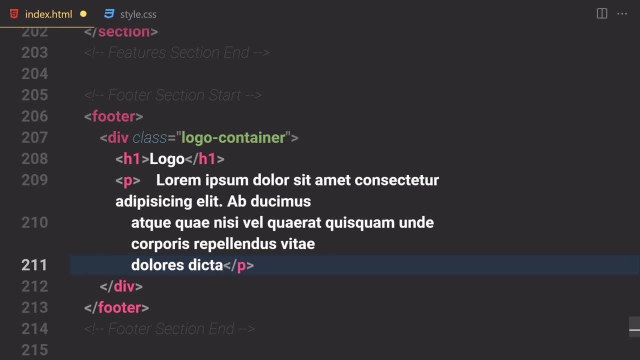 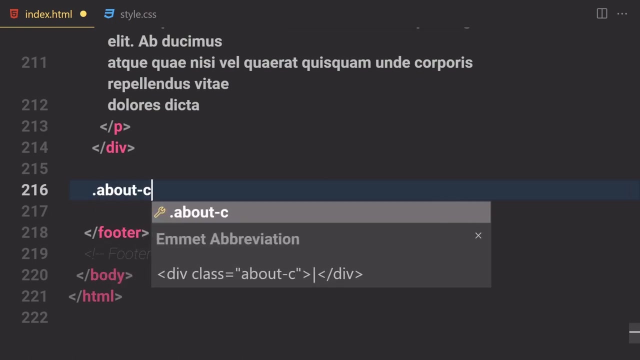 we are going to be using a logo like so and uh, lorem ipsum, of that lot of lorem ipsum, i'm going to copy that from here, come down and paste it right here. okay, so this is going to be our first step. underneath this div we are going to be using, or about company, company like so, and let's just write it with: 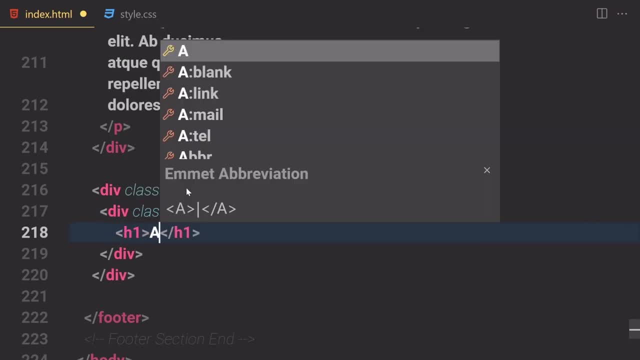 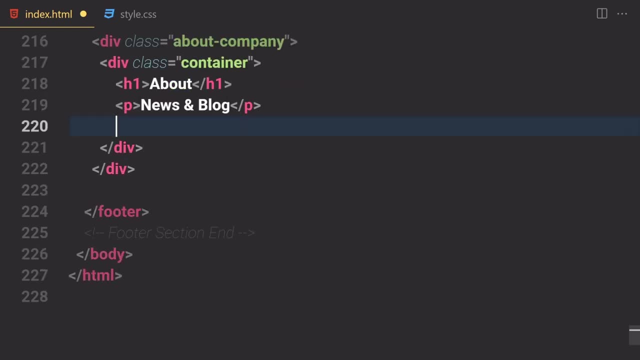 the class of container and let me just write h1 of about in here, and then paragraph of news and block, and let's just write a paragraph of features and paragraph of about us. okay, so in this case i'm going to duplicate this container two times and let's just change this title to be like: 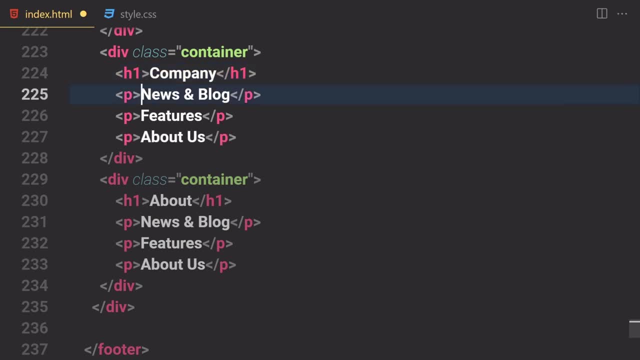 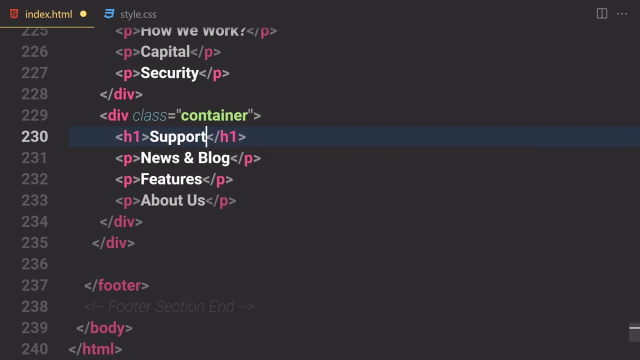 something else maybe, like company, and also this blog and stuff to be, uh, how we work, how we work, question mark. let's just change these features to be capital and also this one to security, this one to support on this one to faq. this faq is okay and then support one more time. 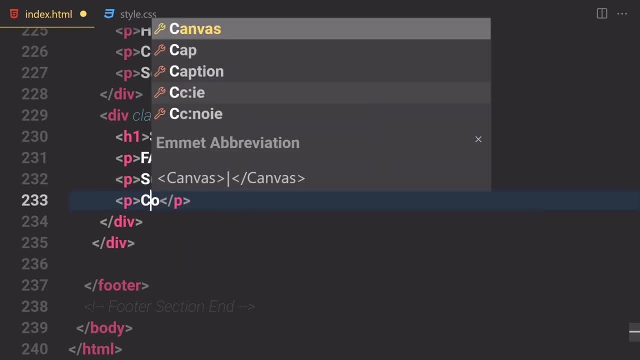 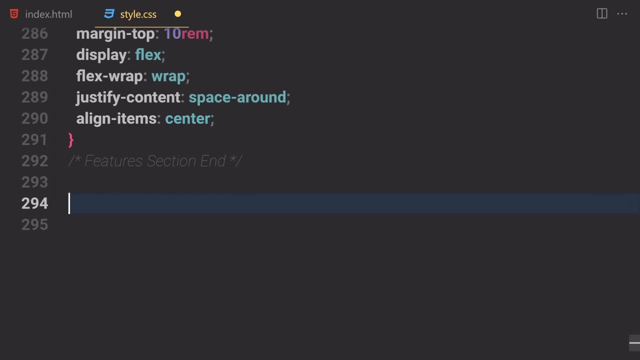 uh, support, and this one will be for contact us. so if you sell that and this is how it looks like. so now let's jump into our css. and now let's just try a little bit. let me just write a four. that's exactly what we are going to do inCBS policy and also when we take a look here in our 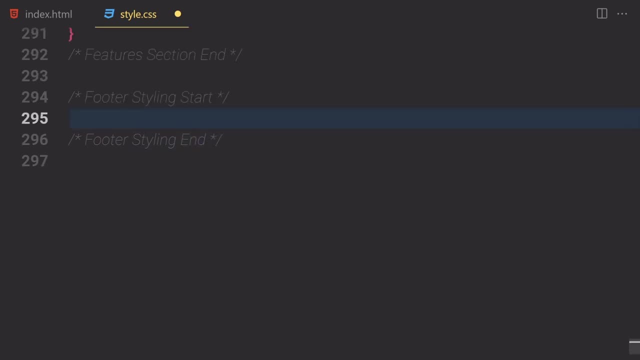 this list. so we have our website. it just we just took a look at the list that we have at the time of duty them. uh, our site질istcom. let's go ahead and press, start, start, duplicate that and this is going to be the end of their styling. let me just get my footer. background of color will be now set to totally primary color and let's just use a margin for the top of 10rem. Display will be totally exposed. muscles will be set to. wrap will be set to lots we have here. 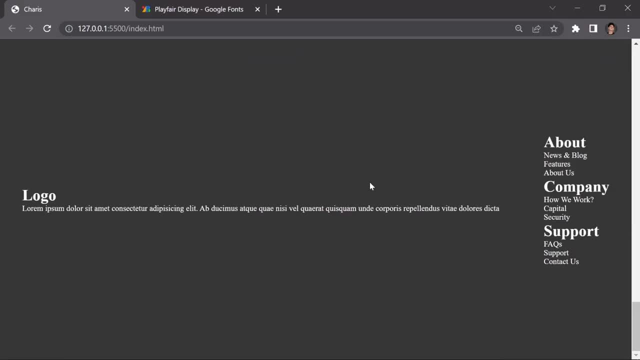 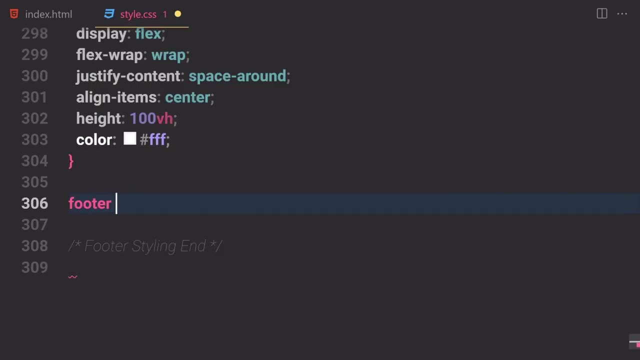 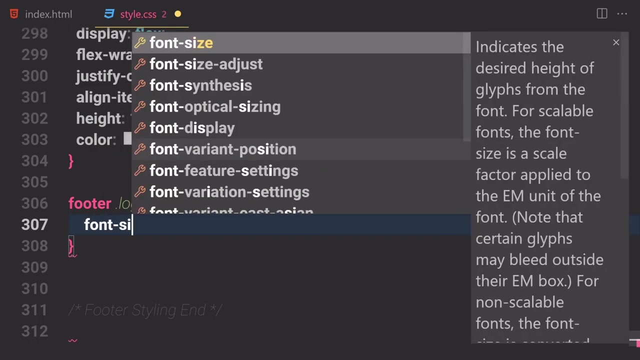 and color will be totally white. so if you save that- and this is how it looks like for now and now, let's just take care of that. um, h1 or footer, uh, then logo container of that h1 and font size, i'm going to increase that to like 4m and the font family will be now set to like. 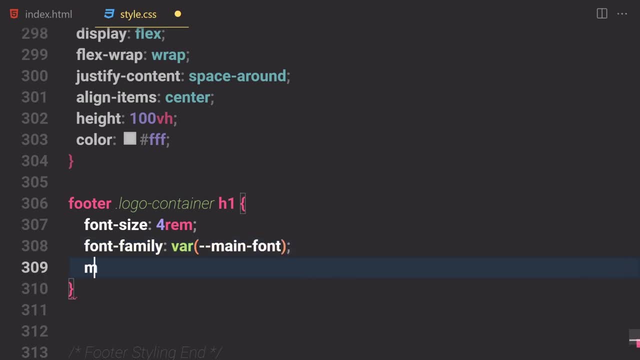 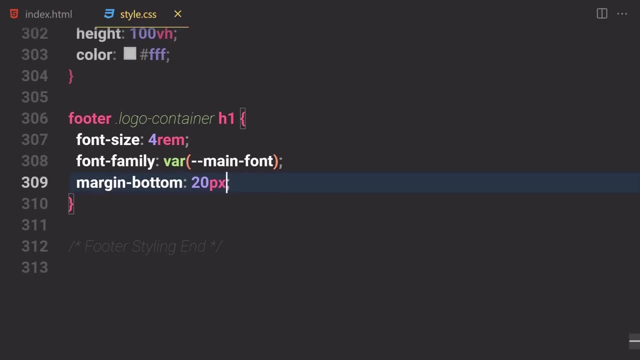 main color- not main color, but main font- and the margin for the bottom. i'm going to give him like 20 pixels. so if you save that- and this is how it looks like right now- okay, so these h1s now let's just take care of that paragraph real quick. so order, and then logo and container. 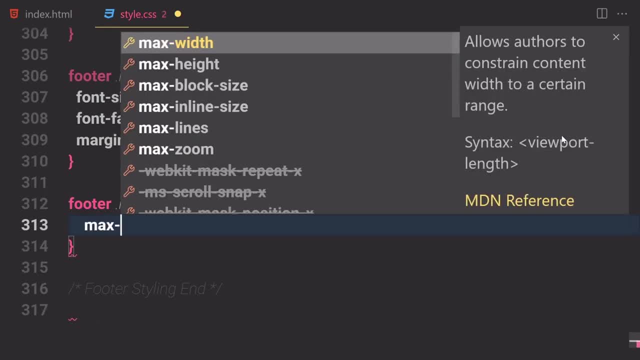 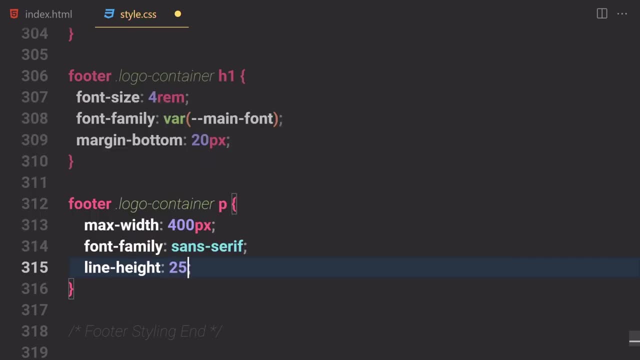 and take that paragraph from there and i'm going to give a max width of like 400 pixel will be fine, and font family will be now set to sensor of line height. i'm going to give like 25 pixels if you save that, and this is how it looks like. so now let's just take care of these. 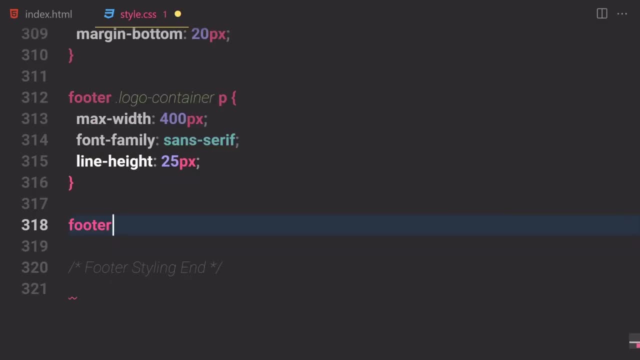 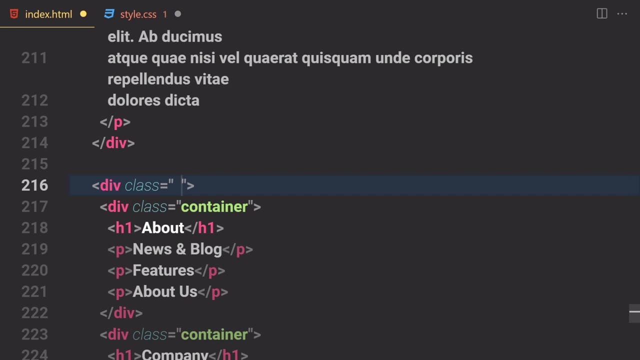 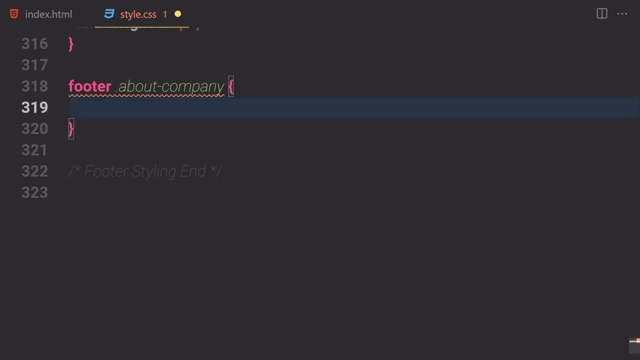 uh, i'm going to write first of all a footer and then about company. so which is about company? let me just copy them. not sure about, uh, if i just type it correctly or not, so i'm going to paste it right here anyways. so let's just write a display of flex on it and flex ramp will be now set. to wrap, and just if i 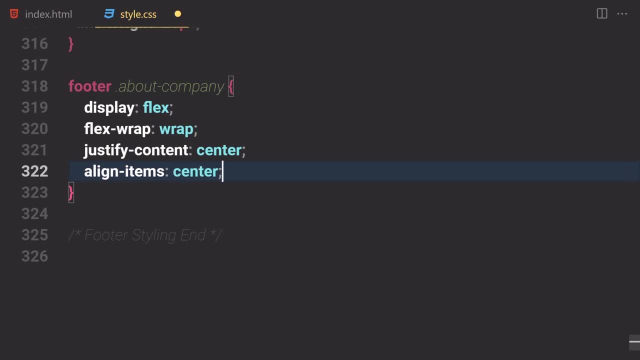 will be now set to totally center. align items will be also set to center. so, if you save that and this is how it looks like, so now let's just probably a bit of spacing in there. i'm going to write about company and then container. uh, just container, okay, so let me just provide a margin. 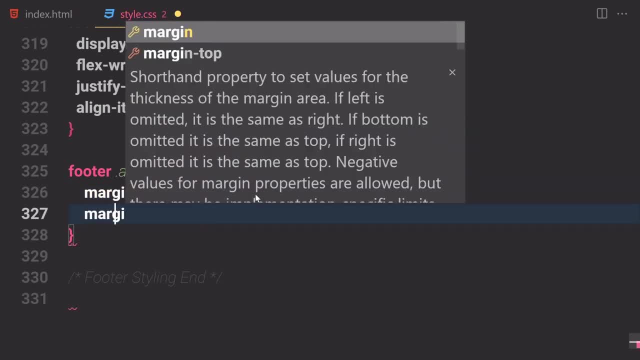 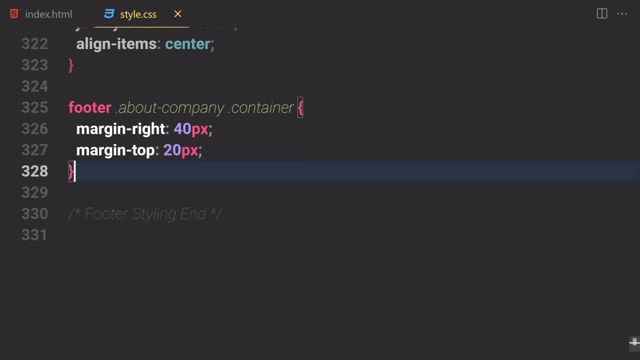 margin for the right will be now set to 40 pixel. margin for the top will be now set to 20 pixel. save that and now we get a little bit of margin in there. so now let's just start working. uh, you know what? let's just probably a bit of spacing inside these h1s and stuff. so 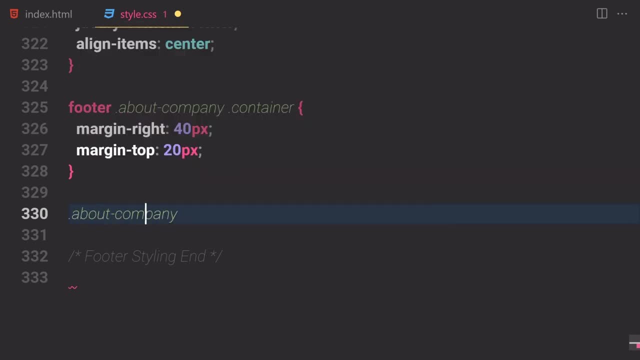 what am i? so i'm going to just write about about company. uh yeah, abo you about company. let's just get our container and h1 and i'm going to give a margin for the bottom of like 50 pixels. if you sell that, that's a little bit of margin, and now let's just use a margin for about company. 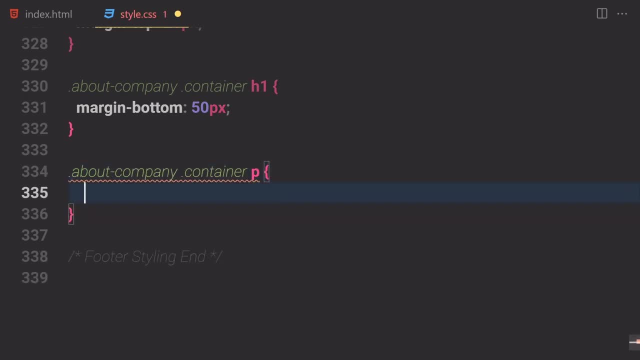 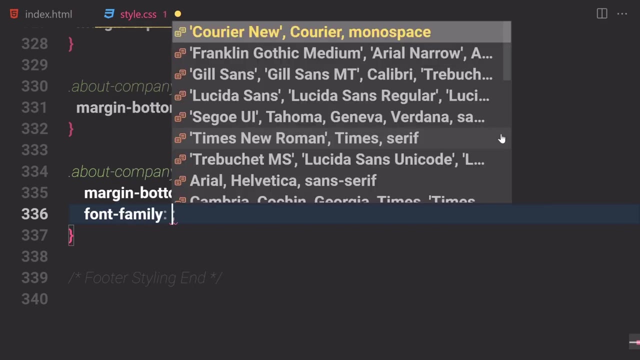 and then container and that paragraph as well. so i'm going to just provide uh word, i'm going to give a margin of like margin bottom of 20 pixel and i'm going to also change the font family to be like sensor. see if you sell that and this is how it looks like right now. okay, so you can play. 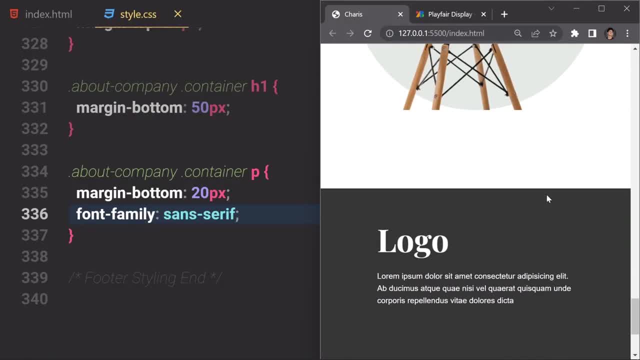 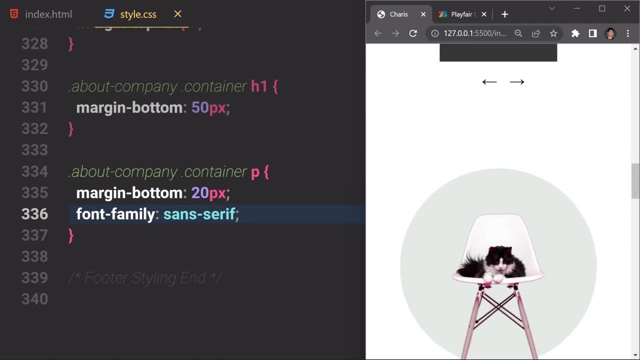 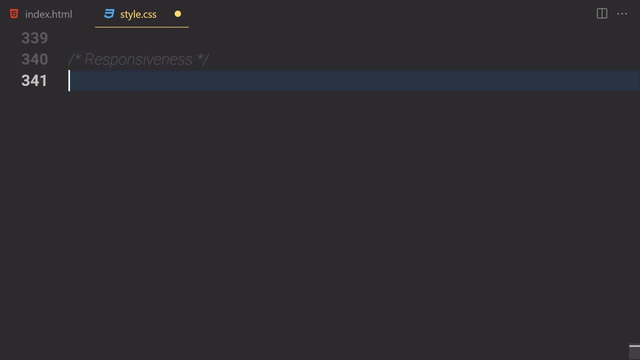 around with that if you want to in your space, but in my case, uh-huh, okay. okay, it's looking cool, but now we have to take care of that by using a or media queries. so now let's just write or responsiveness in here, so responsiveness. i know the spelling is wrong, but i'm not going to waste my time writing a spelling. 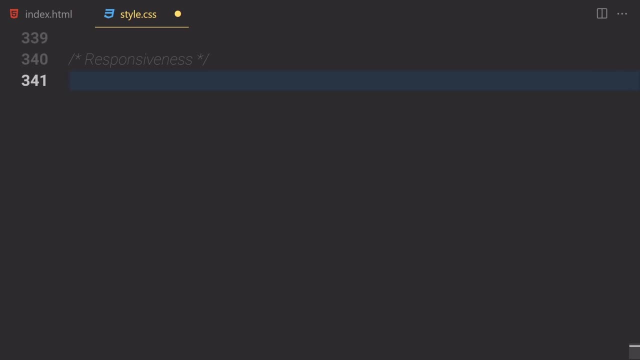 so what do we have to do in this case? let's just start working on our first media queries. i'm going to zoom in a bit and let's just write a media for only a screen and see what we're going to be giving. um, let's just- you can look at this example here. so 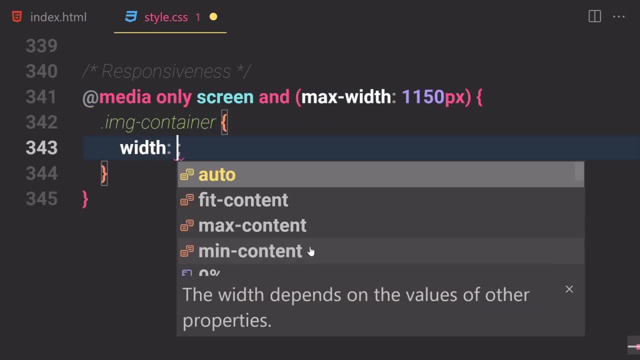 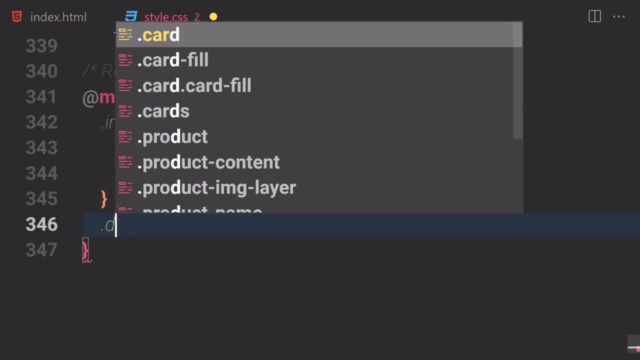 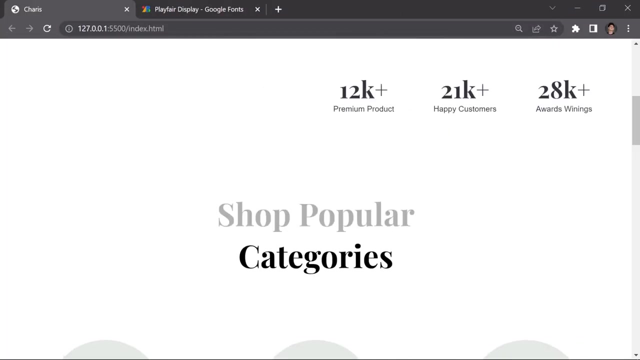 if the max width is what? 1150 pixels. so let's just get our image container first of all, and let's just provide a width of like 340 pixels, and this is going to be it for the height as well, and this d none class which we provide right there. so we are going to be using display of none in. 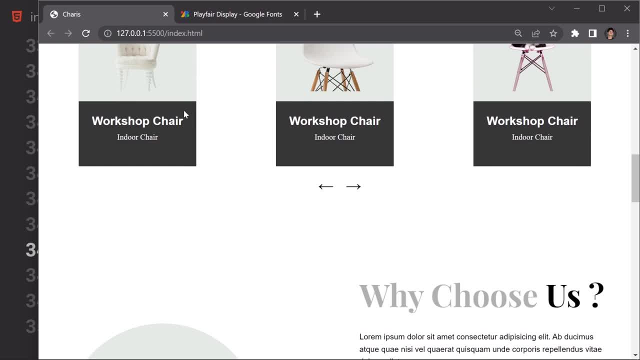 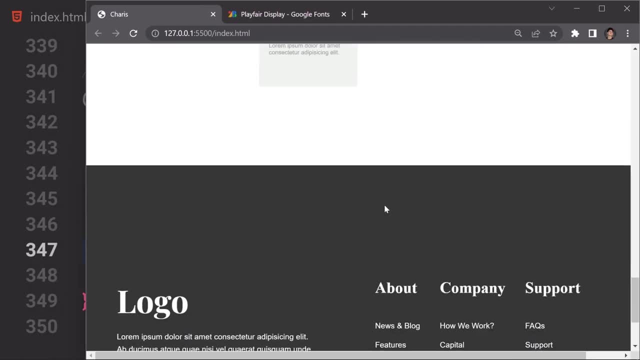 there. so if you sell that and if you make it bigger, like not that much so is working that we expect him to work. and this is gone now i want you to watch this. so if you hit that 1150 and that image will be gone from the viewport right here. okay, so now let's just create. 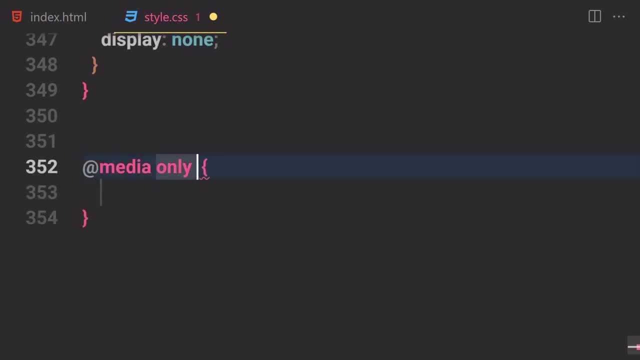 another media query. so let me just write a media only for screen, and the max width is just like 900 pixels. so let's just select our header- a lowercase header in this case, and this is going to be also a px for lowercase. so let's select our header and height will be now set to 120 viewport. 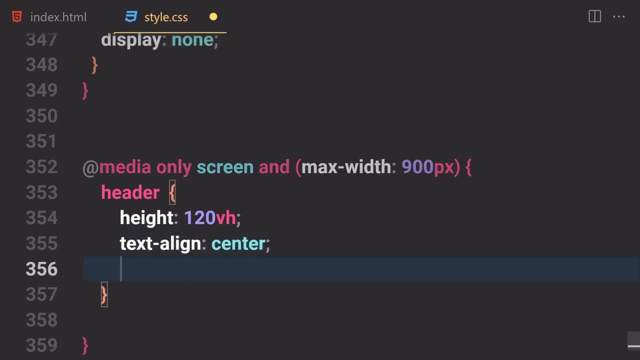 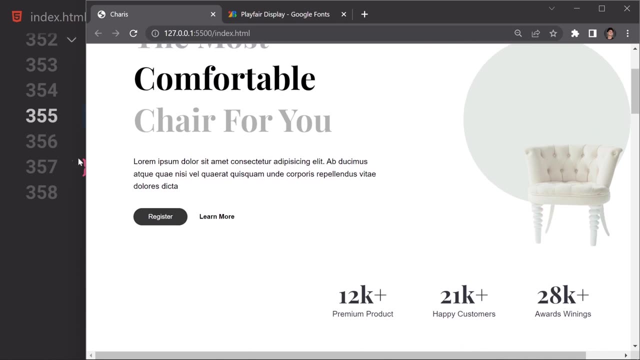 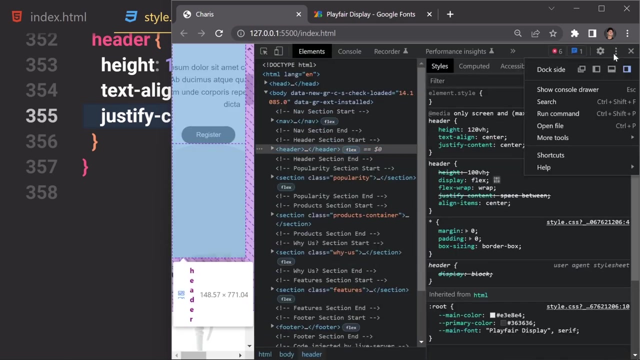 height and text alignment will be now set to totally center justify content. i'm going to give him like center in this case as well. so if you save that, let me just see if you make it a bit smaller. yeah, it will push it right here. so let's just see, right click on it and push that to the. 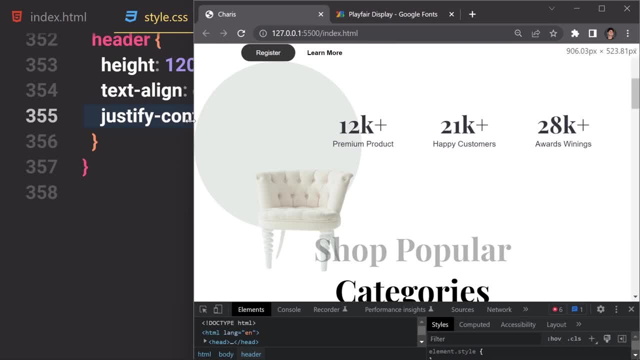 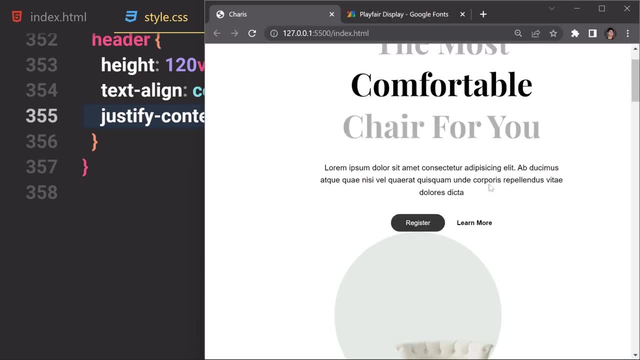 bottom. so if you had like 900 pixel, yeah, yeah, this is how it looks like right now. what else do you have to do? i'm going to cut that from here now. let's just take care of that by using our header content. so let's just select our header. 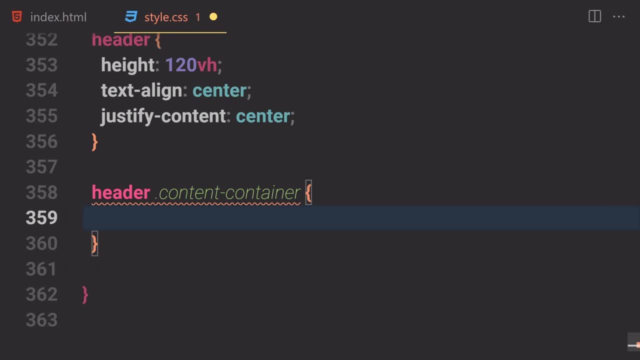 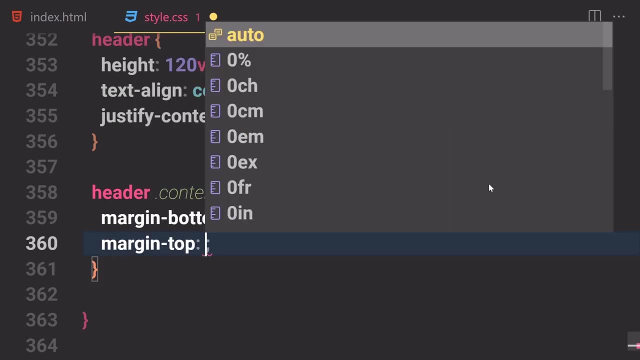 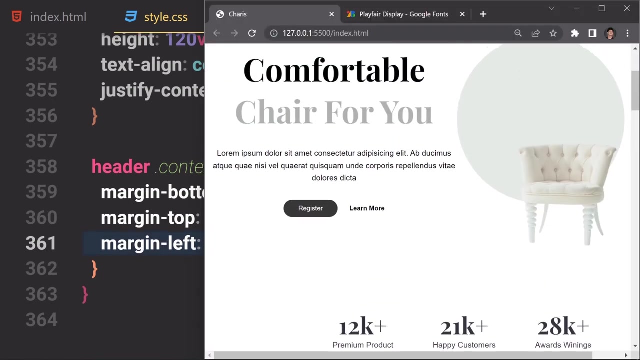 and then content: uh, container. so let me just provide a margin for the bottom, um, margin bottom of sex ram, and margin for the top. i'm going to use like 4m, and margin for the left. i'm going to give him a zero now if you save that, and this is how it looks like right now. okay, so kind of a good to. 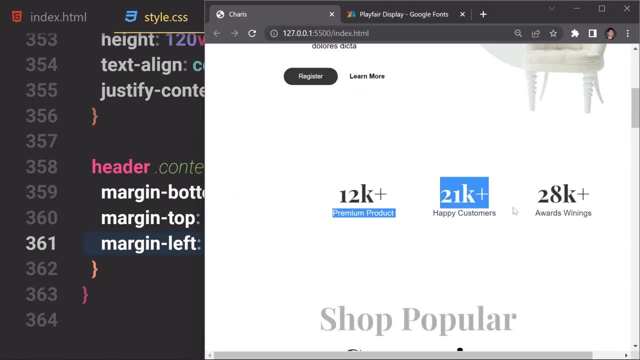 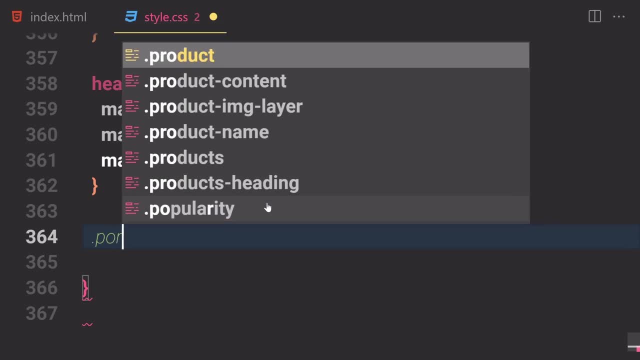 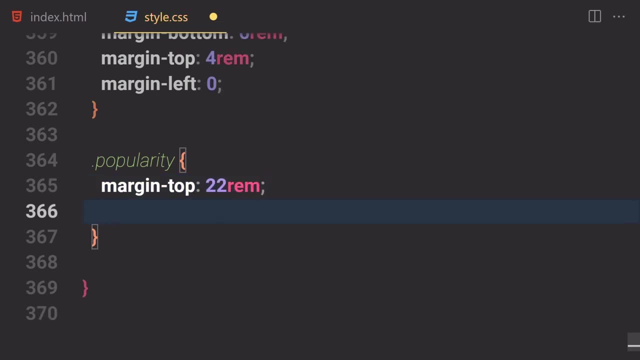 be size. and now let's just take care of that popularity section as well. let me just take care of that real quick. so if i just write a popularity, not product, but p-o-p-u-l-a-r-a-t-y, like so, and i'm going to give a margin for the top to be like 22 rems, kind of a long one, and 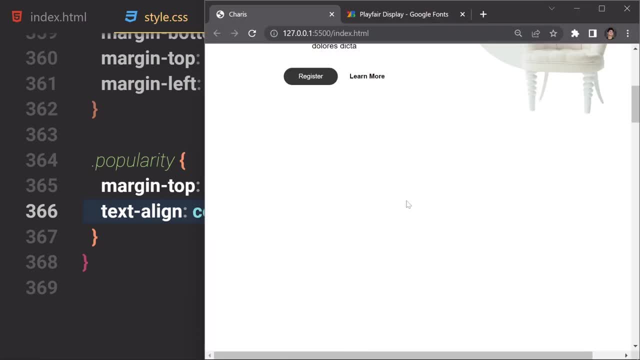 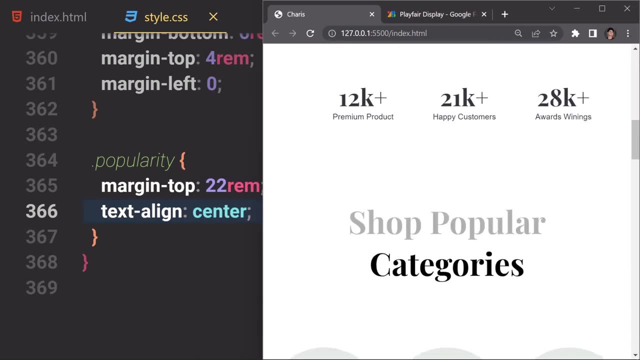 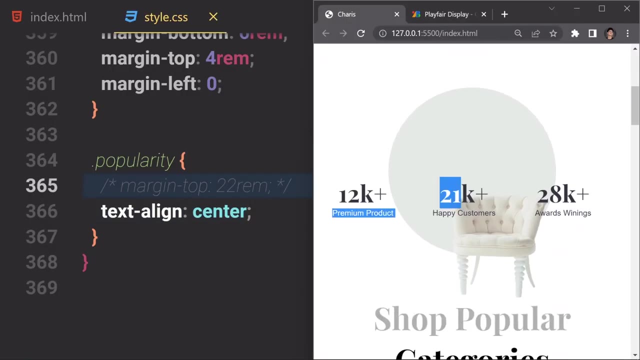 text alignment will be now set to center. so if you save that, and there's a lot of alignment, so yeah, now it's looking better, yeah, that's looking better. so if you just remove that 22 margin and it will not just sponge together right here, we do need that margin for the top. so if you save that, now everything is working. the. 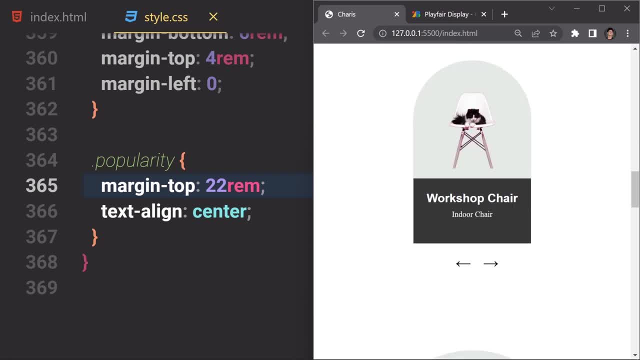 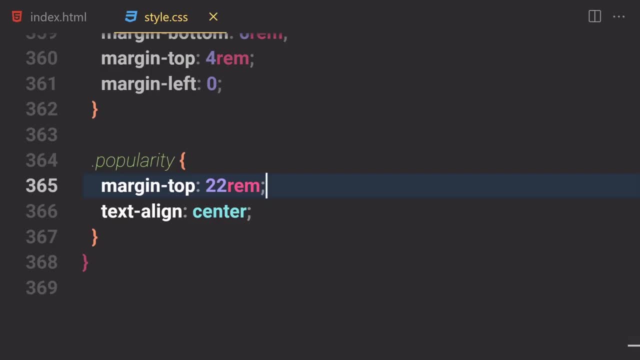 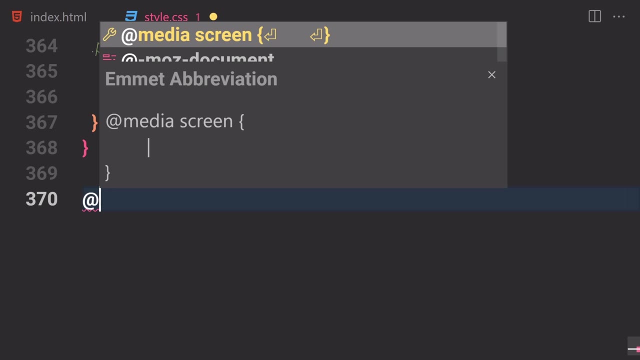 way we expect them to work. so let's just also take care of you don't have for the display of none for this one, because we already take care of that right here inside this media query. to be precise, now let's just write a final media query for a 600 pixel. so media for: 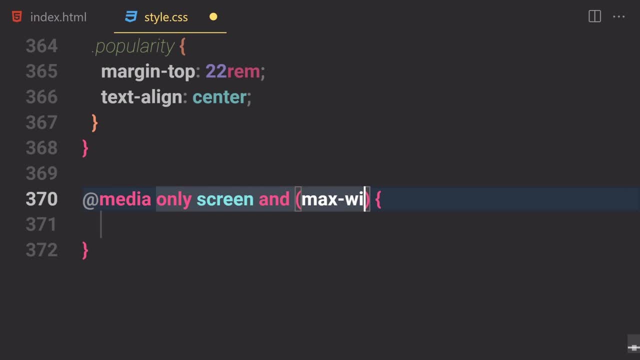 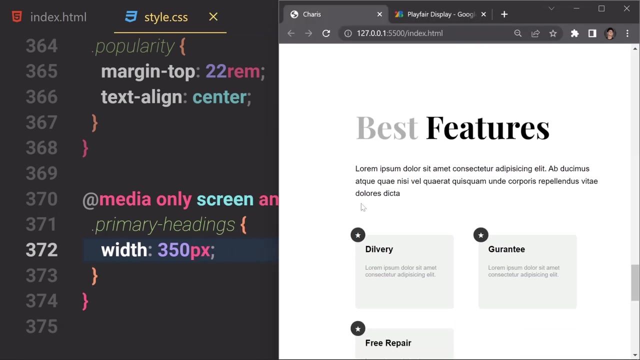 for only screen and for the max width. if the max width is like four, not 400, 600 pixel. so you want to just uh change their primary headings to be like: let me just give a width of like 350 pixels. if you save that now, let's just make that a bit smaller, like so. so it will now take uh that. 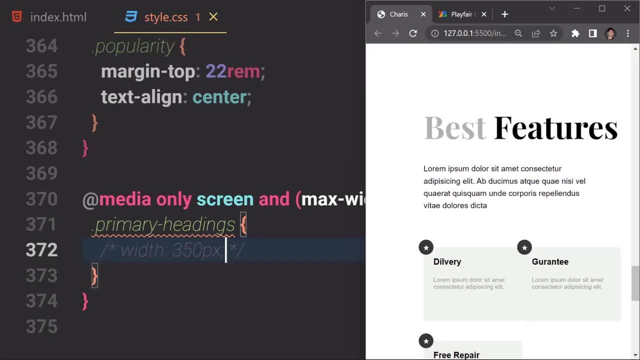 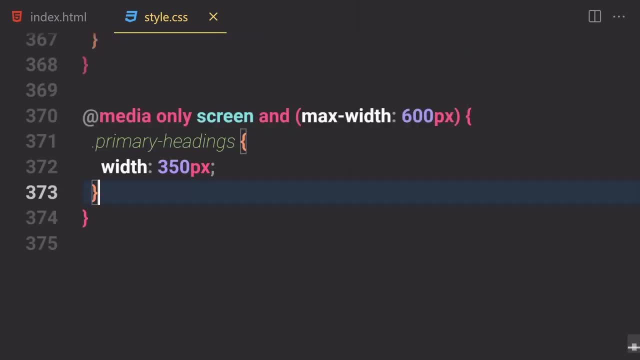 350 pixel right there. so if you just comment out, save it. and if you just uncomment it, and now, if you save that, it'll now just take like 350 pixel of the width anyway. so now let's just take care of the image container. so let me just write img and then container and inside there i'm going to put. 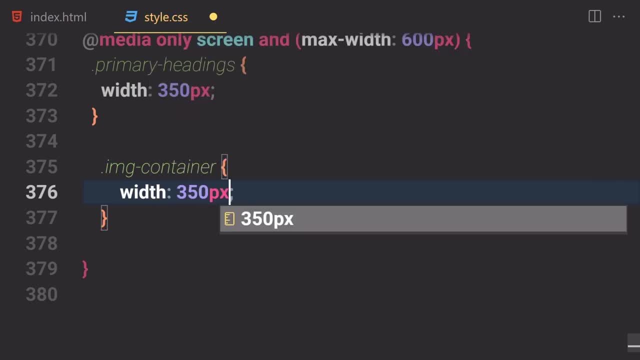 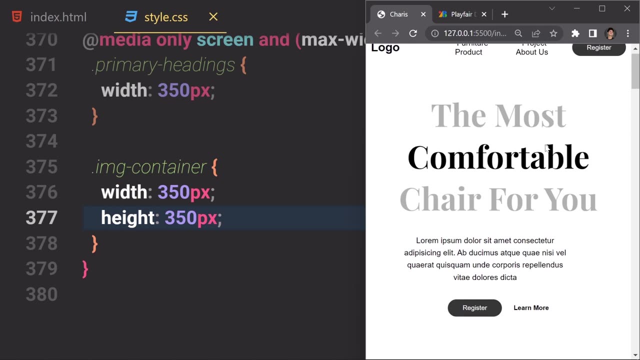 like a width of like 300 pixel- 350 pixel to be precise- and duplicate there, and same will goes for the height as well. so if you save there, so the image container is now totally small right here. okay, so if you just uh comment this line out and if you save there, it's kind of a little bit. 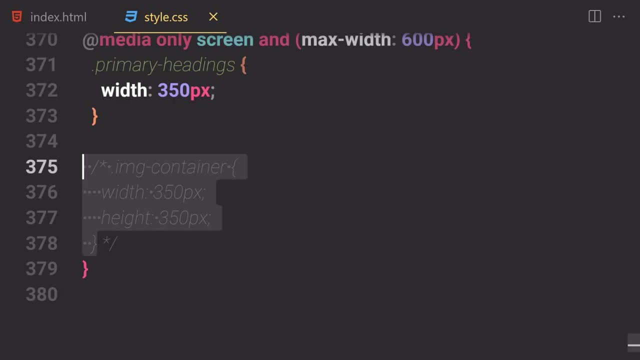 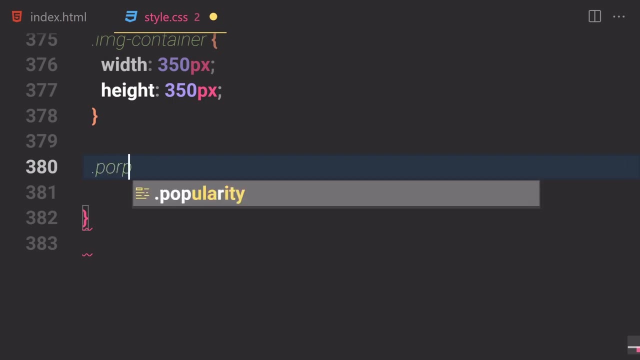 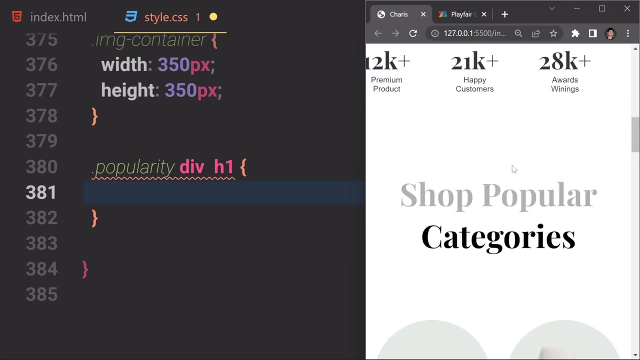 big. you know what that would do, that would do. it's kind of fine, but i'm going to also provide anyways, if you want to play around with that, so you can. and now let's just take care of popular, popular popularity and div, and now h1. so we want to take care of uh, where is our popularity? 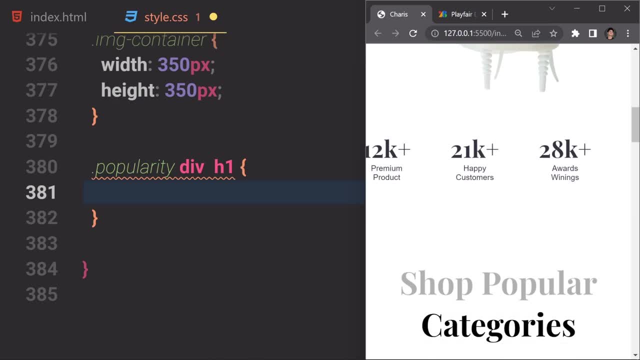 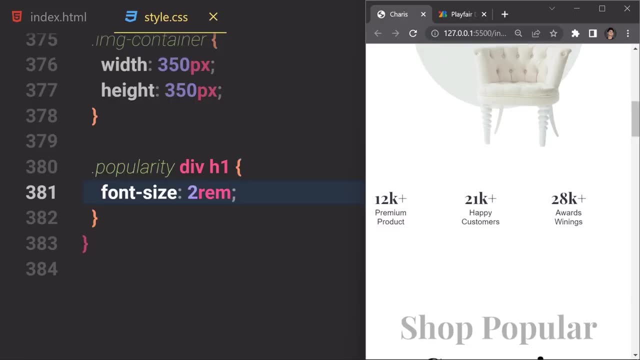 want to take care of that real quick. i'm going to just use like a font size of two grams. so if you save that, and this is how it looks like right now and it's looking better, and now, what else do we have to do now? let's just take care of that popularity div. 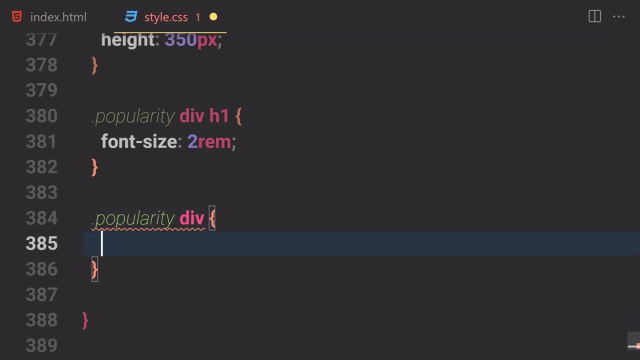 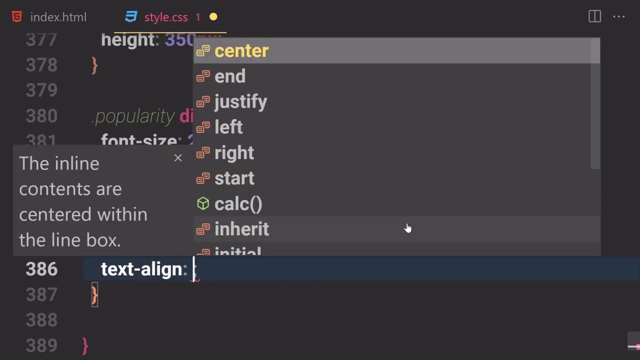 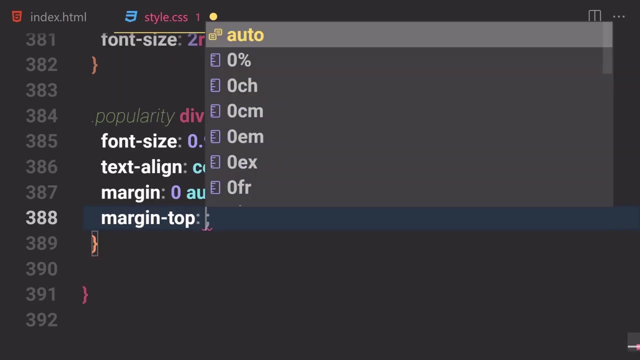 popularity and div. so we have to just provide a font size of like um 0.9 rems. so let's just write a text alignment to be totally centered and also the margin will be zero, auto, so that, so that everything is now totally at the center, and i'm going to also provide a margin for a top. 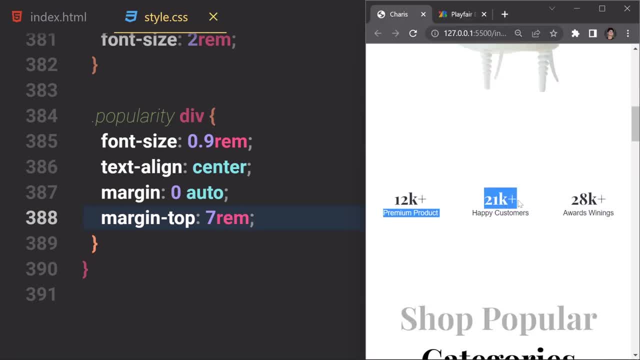 to be like seven rems, so if you save there- and this is how it looks like right now. so popularity section is totally responsive if you want to play around with them anyways. so now let's just take care of our main headings. so these are looking totally big. 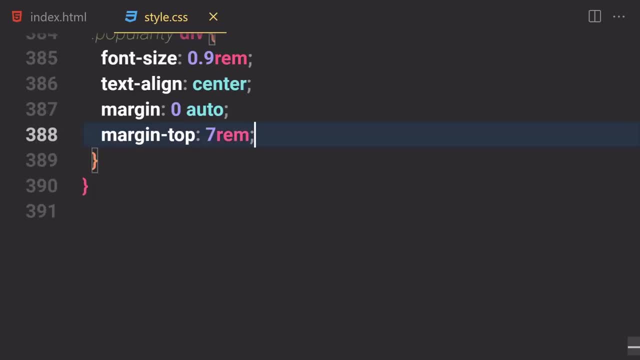 and this one is also looking totally big. so now let's just decrease the sizes of there. so what i'm going to do is that i'm going to just write our main heading, not primary one. come on main headings, let's just select that, and font size will be now three rems. so also text alignment. 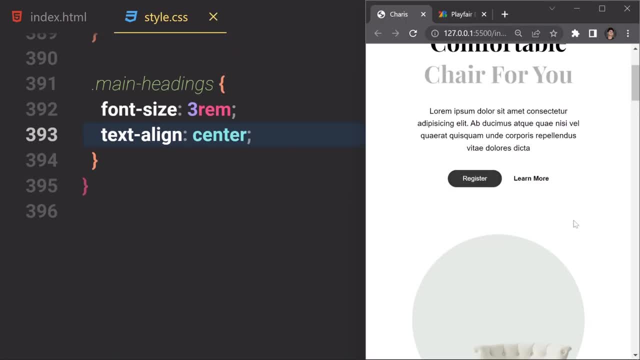 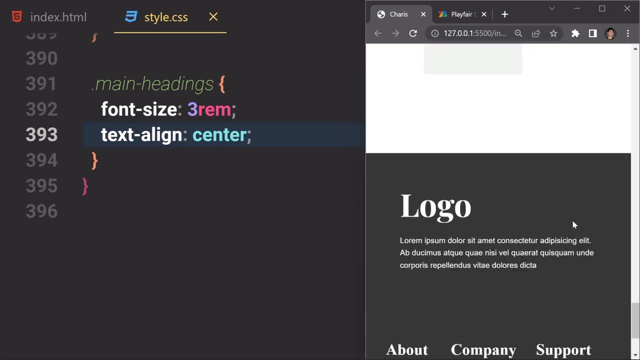 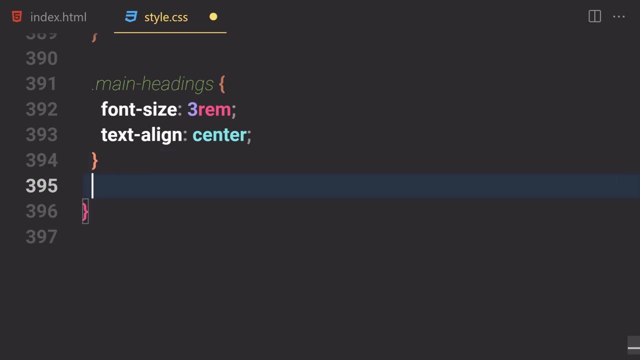 will be set to scenery, okay. so if you save that- and yeah, that's looking totally fine, totally fine, so you can play around with that if you want to, but in my case that's going to be fine, but let's just provide a little bit of margin right on that cards right here. so i'm going to select there real 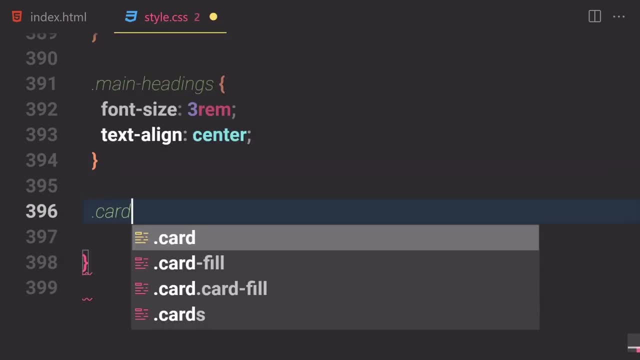 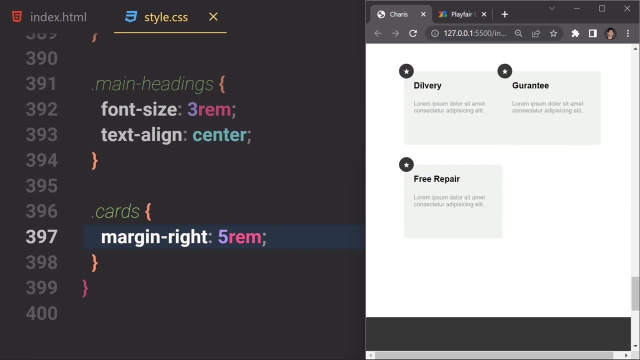 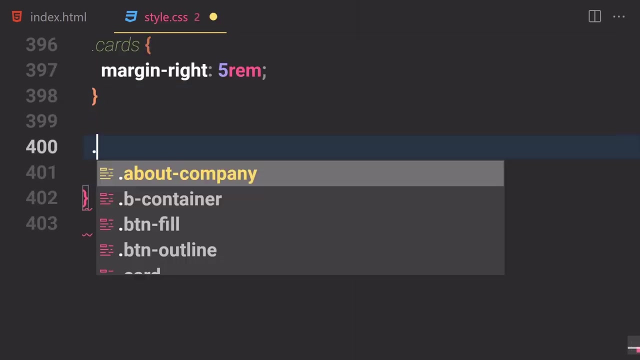 quick uh, what uh cards and margin for the right will be just like five frame would be fine. so if you save that- and now they're looking totally cool, and also for the uh, fill these on as well. so now let's just take care of that, and this is going to be our final step for this project, so let's just 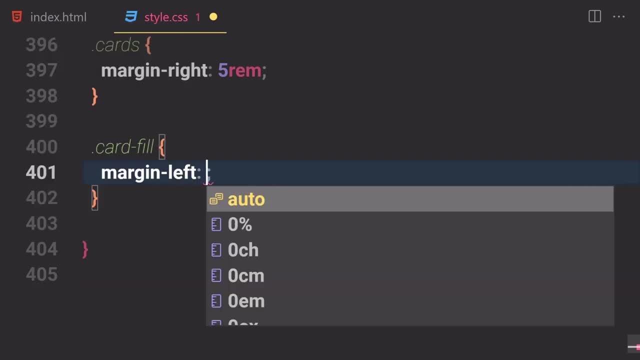 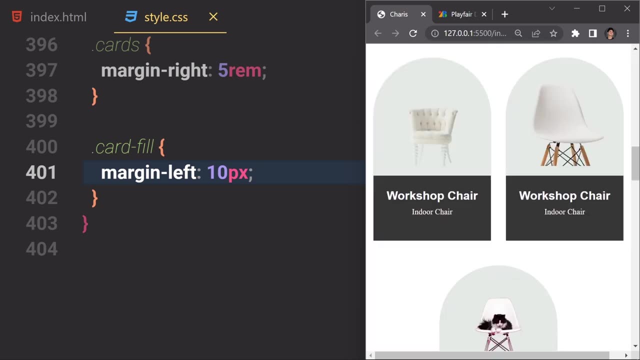 so car fill and margin for the left. i'm going to give them like 10 pixels if you save that, and yeah, they are looking totally gorgeous anyways. so congratulations, and we are now totally done with our project. we make it bigger, and this is how it looks like on a bigger screen. 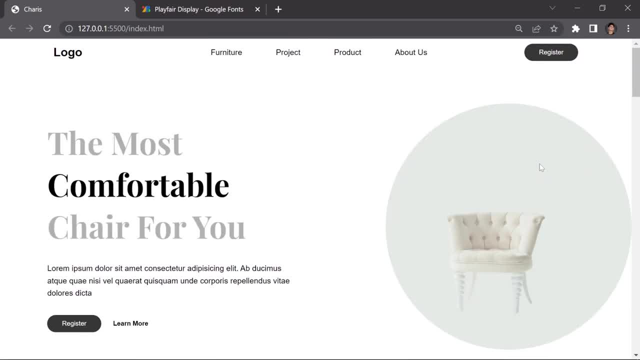 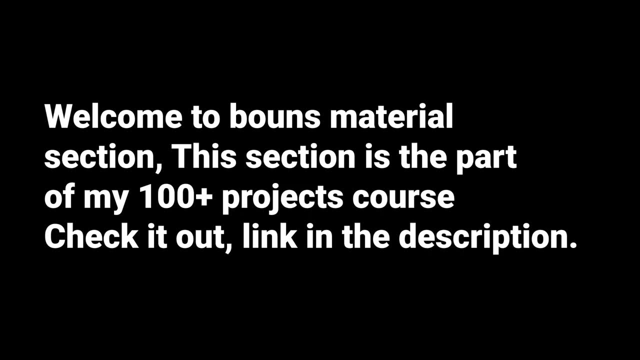 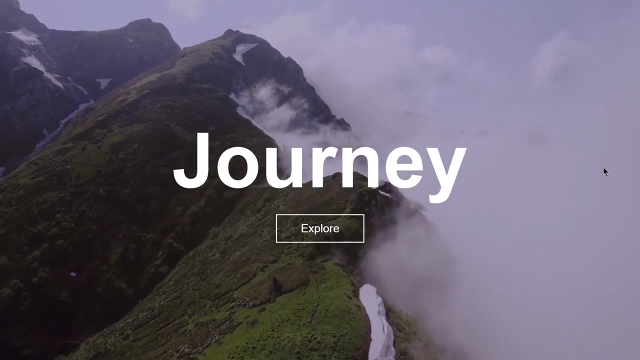 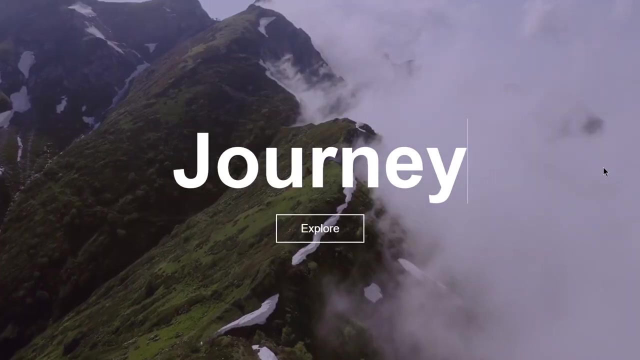 and you already saw on a smaller screen. we are now totally done with this project, so i will see you in the next video. bye, hey guys, hussein, and welcome to the first project of this course. so in this video, we are going to be learning about how you can create a background video by just using html and css. so this is what. 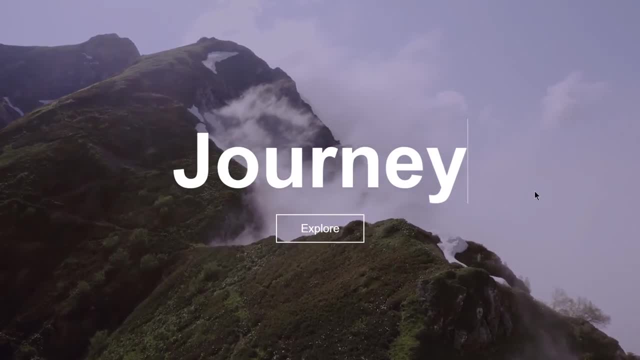 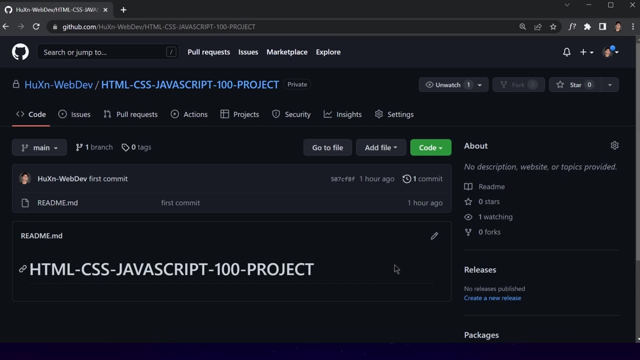 we are going to be building in this video, so now let's jump right into the code editor and write our code. in the previous video, we've made a set of our recording journey. in this video we are going to be creating our first project, which is how we can add a background video by using just html and 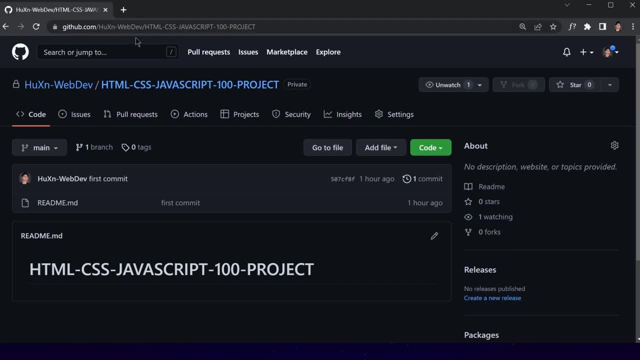 css. okay, so we've made a set of our recording journey and we are going to be creating our first project, which is how we can add a background video by using just html and css. okay, so we've created the github repository right here and we also create this folder right here. but now what? 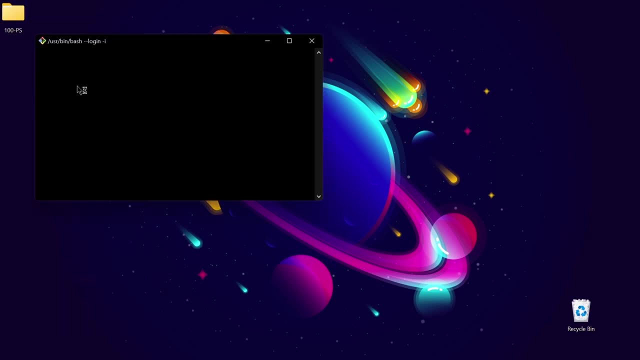 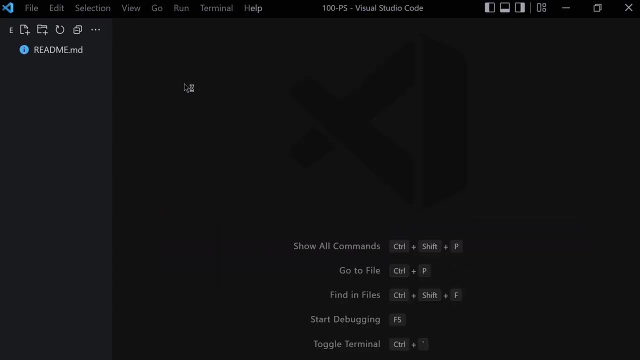 i'm going to have to do now. i'm going to right click on it and then click on get bash here, and then i'll just write code and dot and once i hit enter right now, so it will automatically launch your visual story coder for us. okay. so then i'll remove this um terminal from there and then i'll. 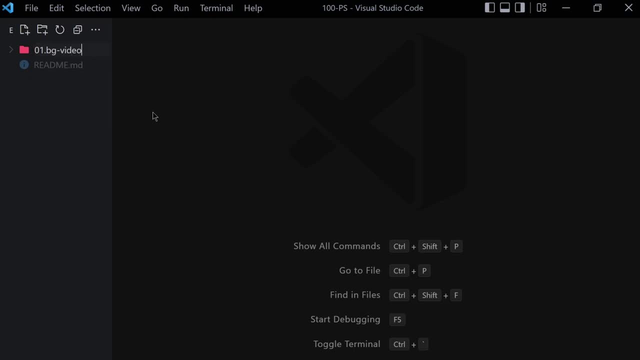 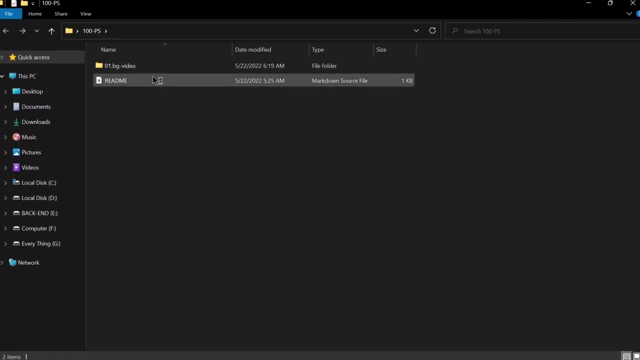 create a new folder given name of 01.bg video. okay, and i guess that will be fine. and if i hit right now, then inside this folder i want to create two files and the first name will be indexhtml and the second one will be stylecss. okay, so now i'm gonna just pass this video, right. 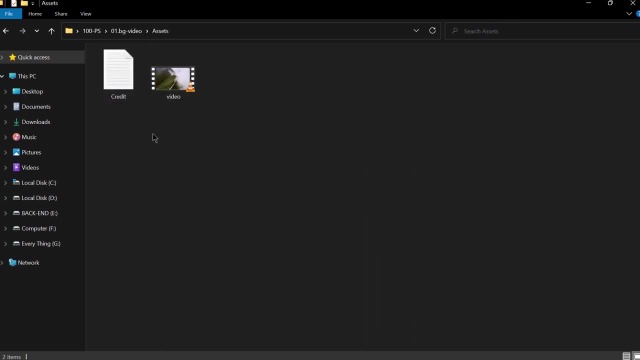 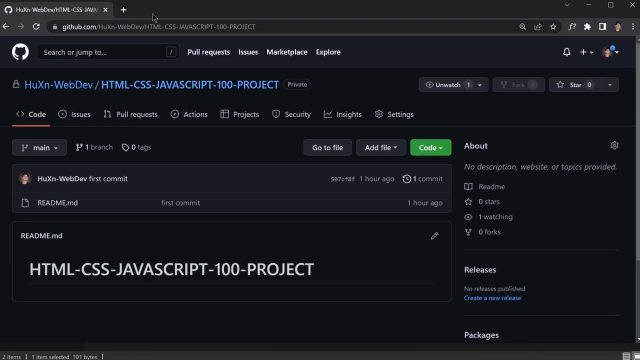 here because i've already downloaded this video. but if you guys didn't download this video, so i'll also provide the link, uh, in the description area, so you can click on that link and it will bring you to this page right here, this video page right here, so you can download from there and by. 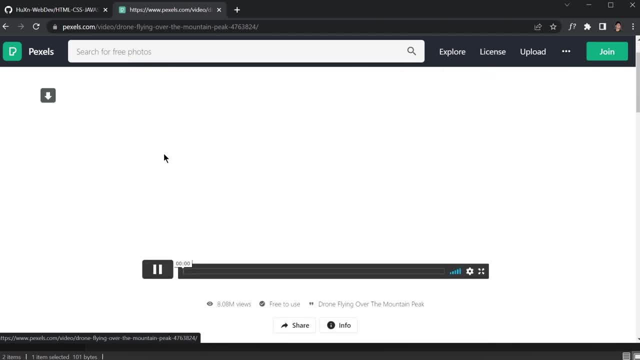 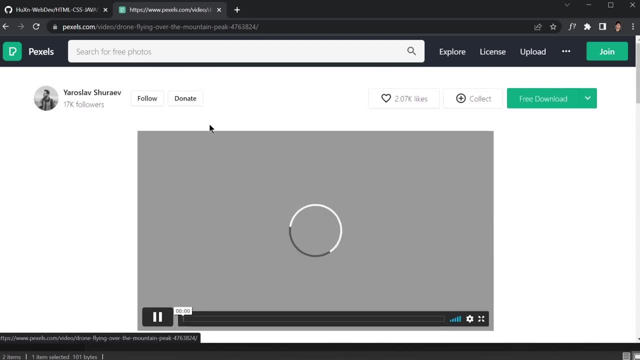 the way. shout out to this person. i can't pronounce his name, but you can just click on this free download and it will start downloading. okay, so it's free to use. so that's why i'm using this video right now. all right, and now we are good to go. so here you can see, we have this assets folder. 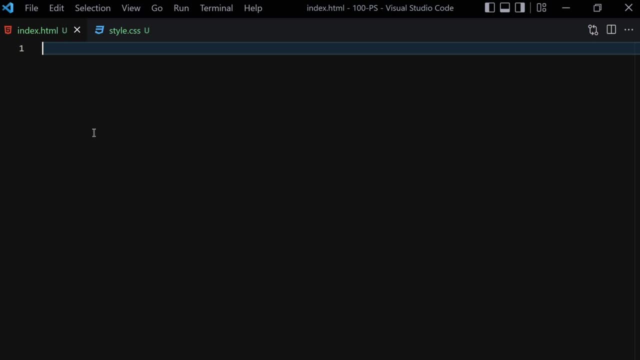 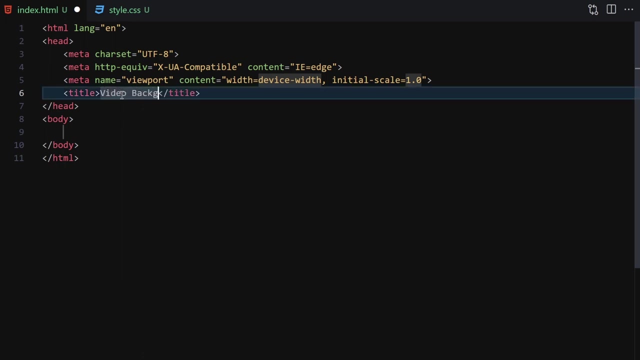 it should be a lowercase. as it's not uppercase, okay, and then i'll also hide the sidebar, or you know, yeah, i'll just go with that. and then i'll just write like doc, and if i hit tab right here, so it will create or boilerplate right here, and then i'll just write like: uh, where do you background? 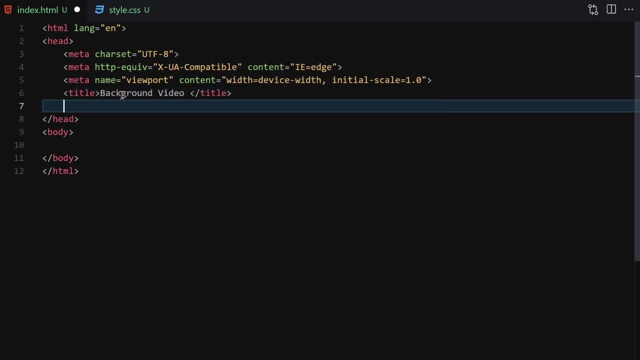 or you know our background, where you will be, fine, you, and then i'll link my css really quickly right here and we don't have any scripts, so we are not going to be providing any scripts, so i'll just save this file and then i'll right click on it. 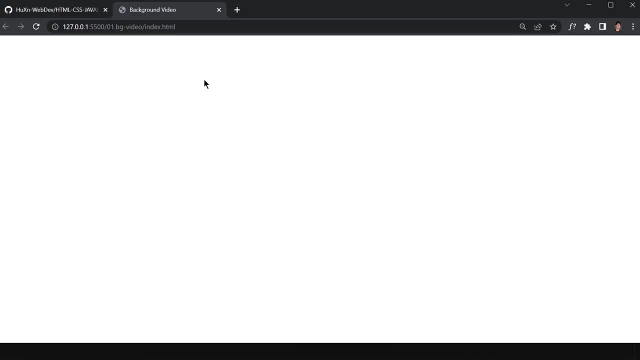 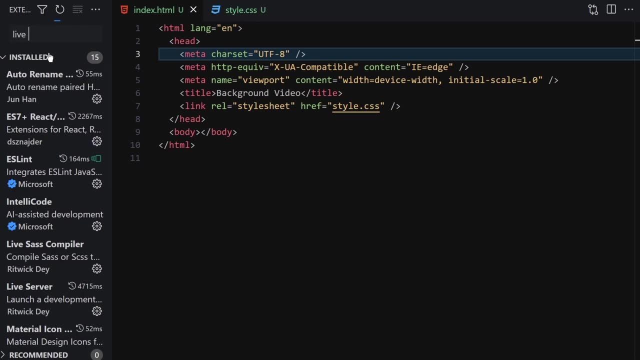 and then click on this: open with live server. so if you already installed live server, so it will open it for you. if you didn't install a live server, so go to your extensions and then just write like live server, server and then click on the first one and then just download it. so here. 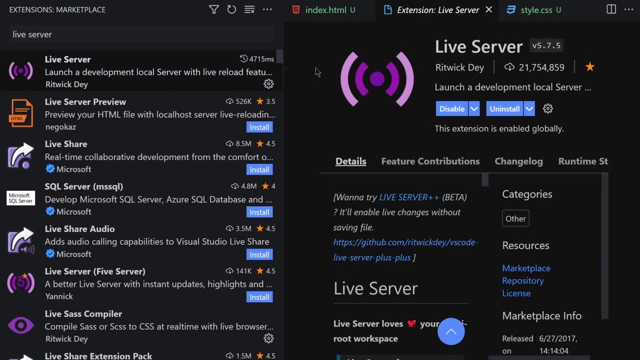 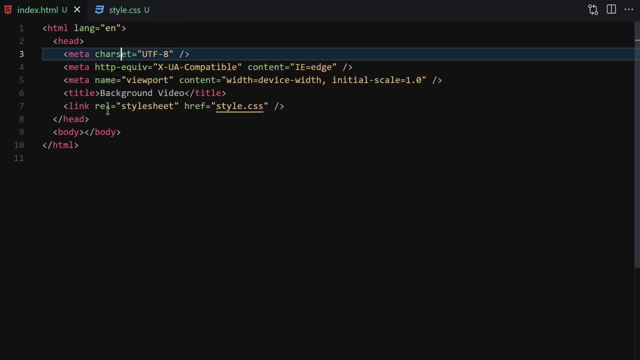 you can see if i can make it. so then click on this live server and then just click on the install, and here you can see i've already installed it, so i shouldn't have to install it, reinstall it again. okay, so now i'll hide this. metas and head data from now. 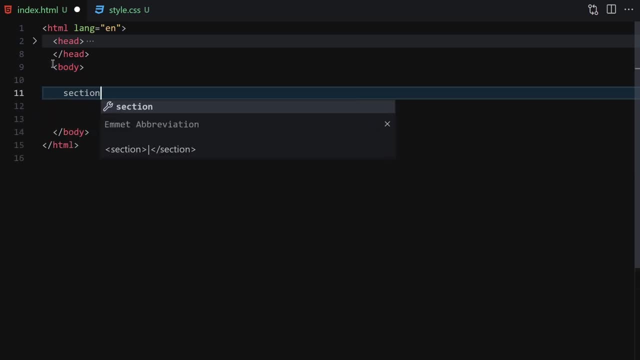 and now the first thing i'll do is that i'll just create a section and give a class of hero. right here inside this hero class, we are going to have to provide first of all the video. so i'll just write like: um, where do you here, or just where you would be fine, or you know, i'll just remove this. 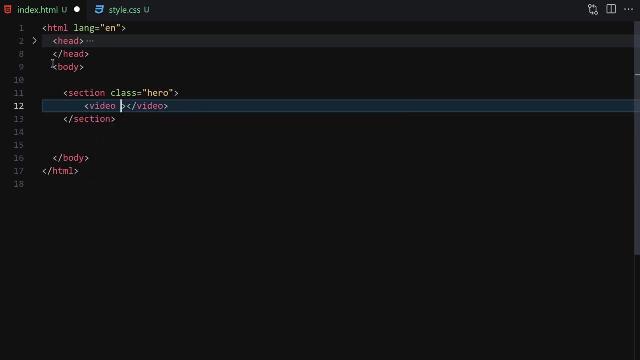 comment, because we are going to be writing our video right here and then i'll just create a section. source will be outside, so we will just provide like a source of um src. and then i want to hit control and space and here you can see we have our assets folder. because we have this assets folder, 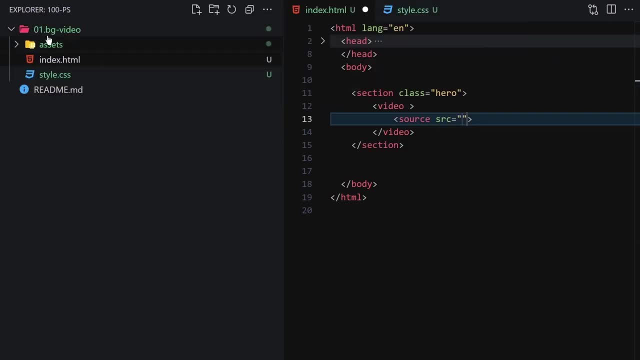 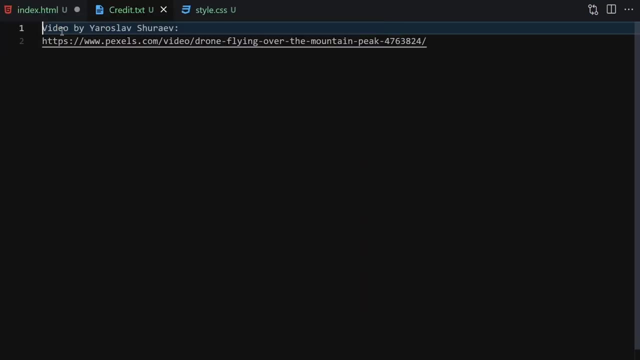 right here. so inside we are now inside this bg radio. inside this bg radio folder we have this assets folder. inside this assets folder we have this credit of this video. like the guy name is this one, and here is the link: um of the video. so if you want to download it for yourself, 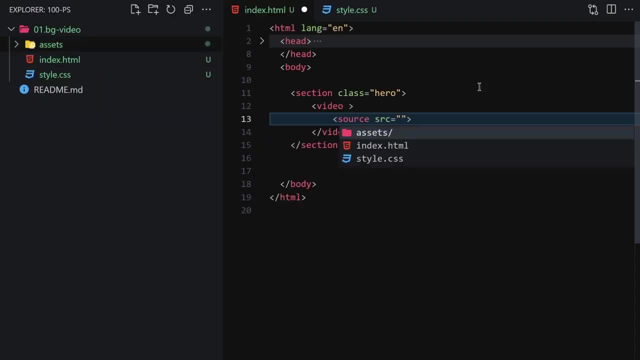 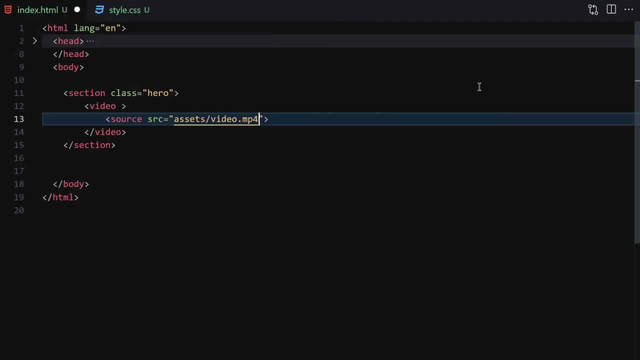 and here is the video. okay, then i want to hit control and space and go to the assets folder. inside this assets folder i want to go with: uh, this video okay, and then i'll collapse my sidebar one more time and save it, okay. so here now for this video. i'll provide a few attributes. the 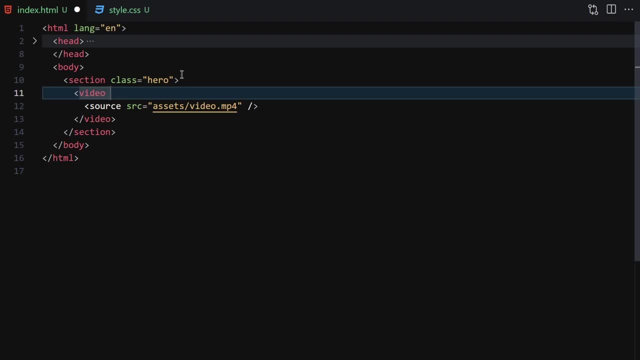 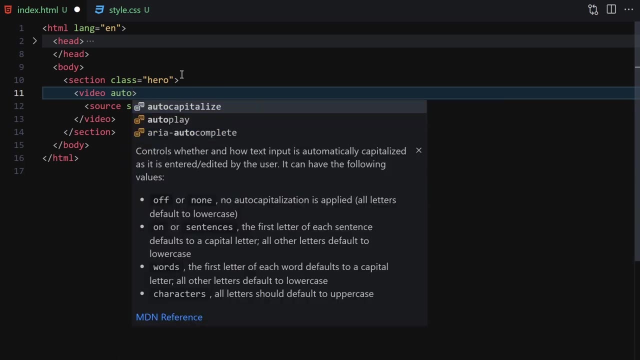 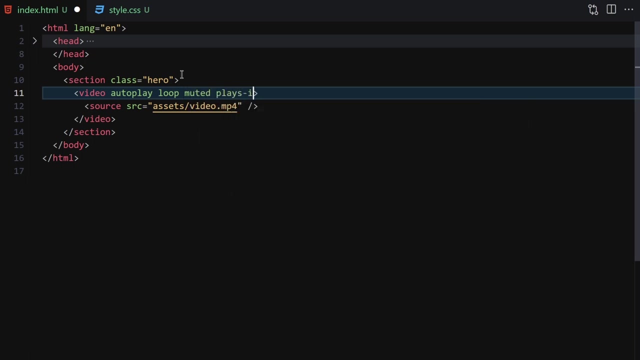 first one will be autoplay, not optimize all sorts- uh, i don't know what their type. so just write like auto play, come on autoplay. and the second one will be, and the third one will be muted, and then i'll just write like players in line and i'll also. 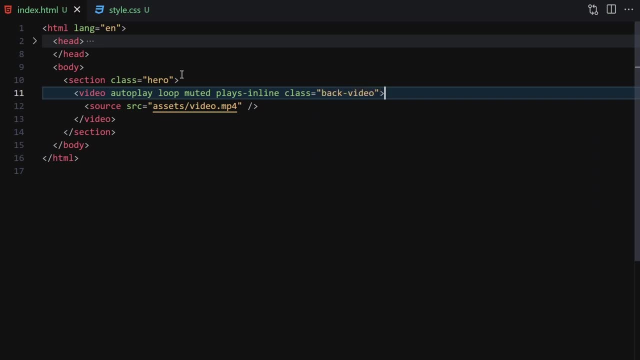 give my class of like back video. okay, so once we set our file inside this hero section, we are going to be just right underneath the video we're going to be providing the content section. so i'll just write a section and give a name of like- not name but class of content- and inside this content, 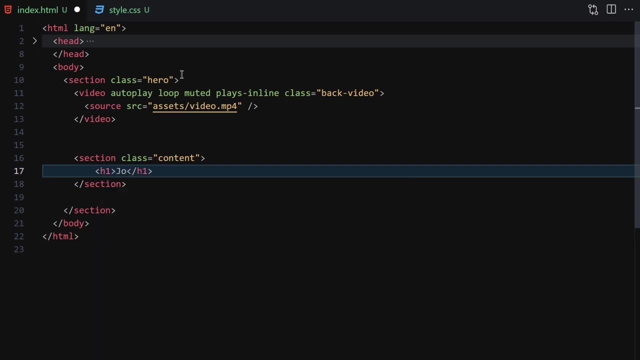 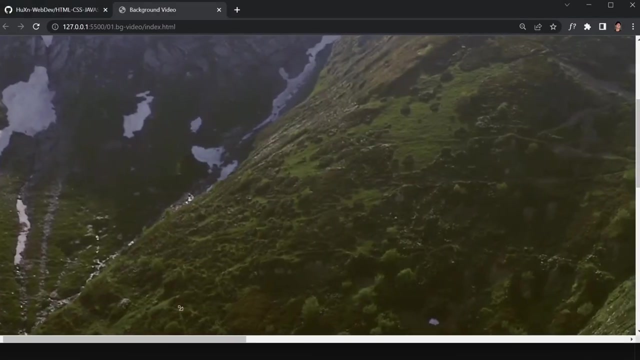 section i'll write like h1 of journey or you can write any text you like, but in my case i'll just write like journey. yeah, i did, and then i'll just write like anchor tag and it will go nowhere and i'll just try to explore. okay, so once we set our file, so here you can see, we have our video right here and here you. 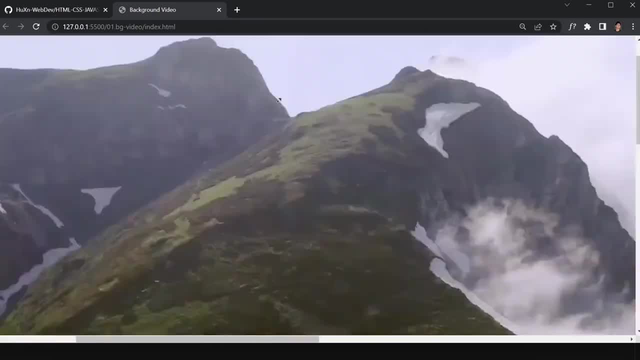 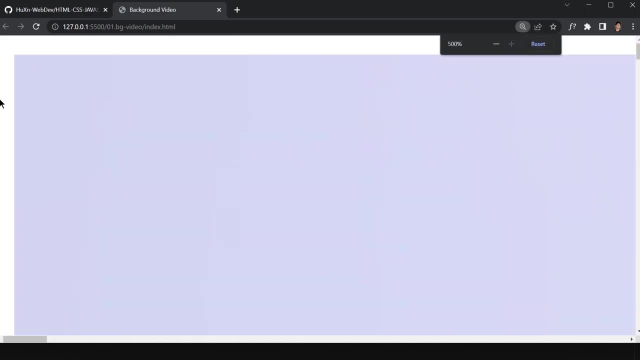 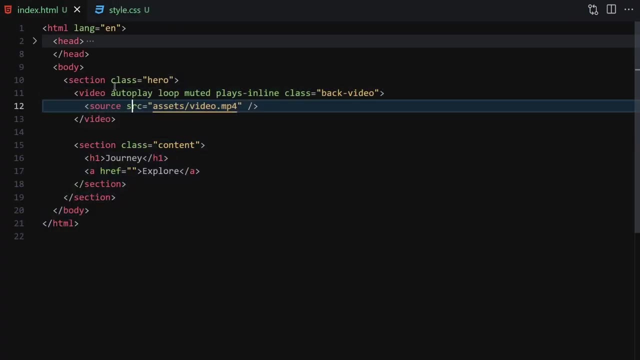 can see. we have our text right here. okay, no styling whatsoever. it's looking ugly, all right. so the first thing i'll do is that i'll remove these empty spaces from here. like here, you can see these empty spaces. so for that we have to write our resets, so i'll just go to my css file. yeah, i'll link it and 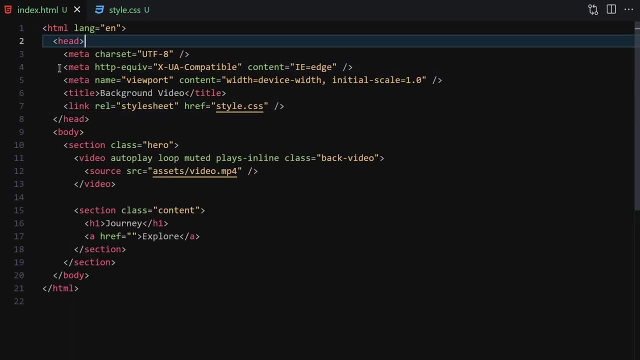 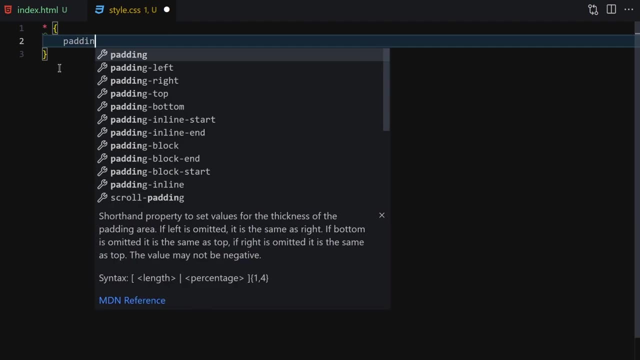 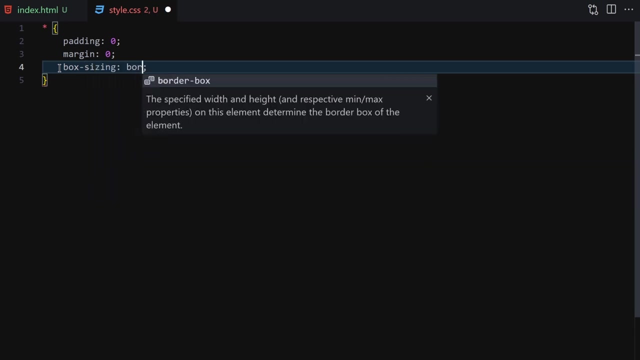 i guess i, yeah, i link it right here. so i'll just collapse this meta from now and then i'll go to my css file and the first thing, i'll just select everything and i'll provide a padding of zero and then margin of zero, box sizing. sizing will be poor box and font family will be sent. serve. 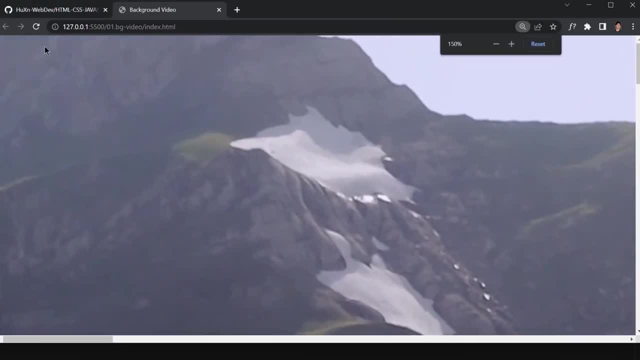 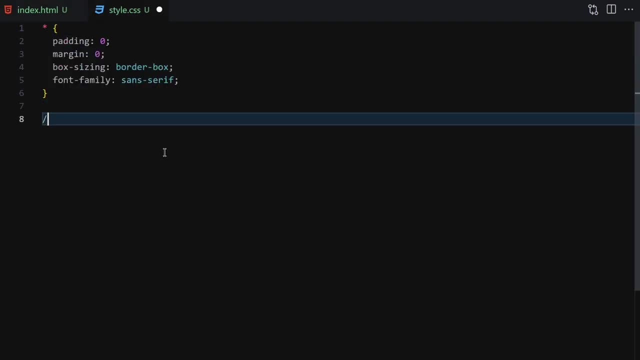 okay, and once we set our file- so here you can see- their empty space is gone. all right, so the first thing i'll do is i'm going to select this hero. right now i'll just write hero and then i'll write a width of 100 percent and height of 100 vh, and once you set our file, so everything is 100. 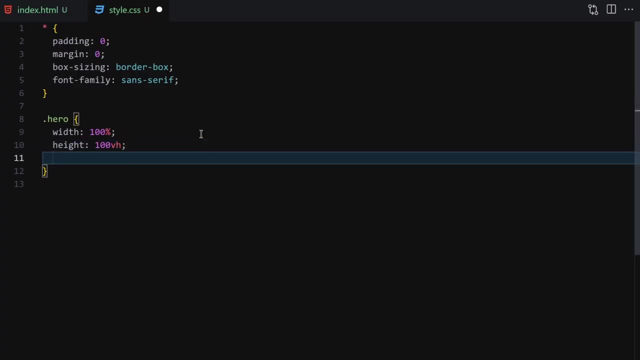 by 100. okay, and the next thing i'll do is i'll just provide a linear gradient, so i'll just write like bg image, or you can also just write like a background if you want to, but their background image will be a little bit precise. and then i'll just write like a linear gradient. okay, and the 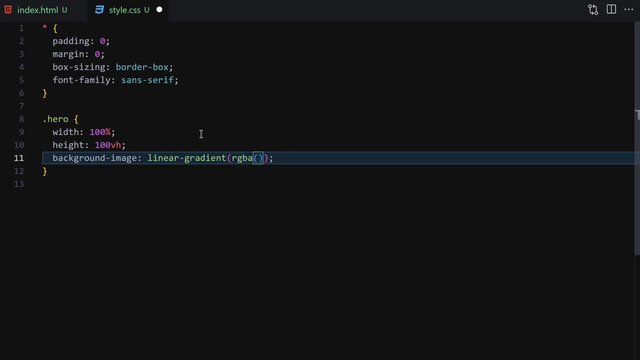 first, linear gradient. i want to provide a background image, so i'll just write like a is like ogba 12, and then 3 comma, uh, 51 comma, 0.3. okay, one, three. then i'll copy this from here and i'll also provide a comma right there and i'm going to paste one more time. 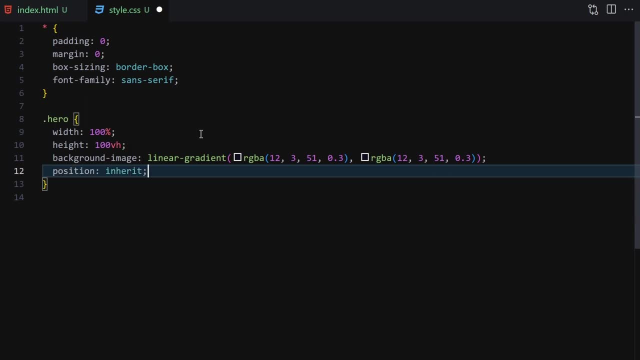 okay, so this is our linear gradient, and then i'll just write a position to relative, then i'll write a padding of zero and five percent and then display will be four. flex, justify counter will be center, align items will be also center. once we sell a file and we 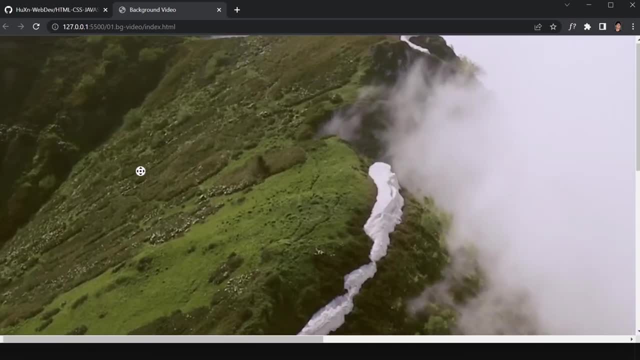 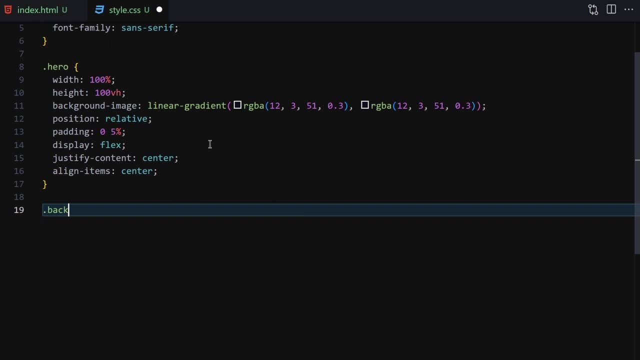 will still see nothing right here, because we can perfectly center this video. so now let's do that. the next thing i'll style is this back video really quickly, so i'll just write like back and then video: okay, and then inside this back video i'm going to just write like position. 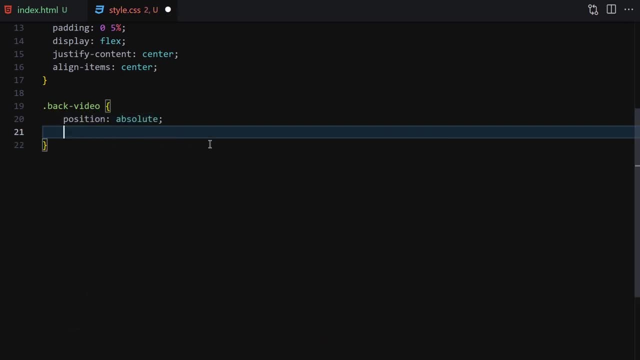 position of absolute, and then right will be zero, bottom will be zero and z index will be minus one. and once we sell a file, so here you can see, our text is now perfectly centered in this video or in this background right here. okay, so now let's style this uh text in this tube right now. 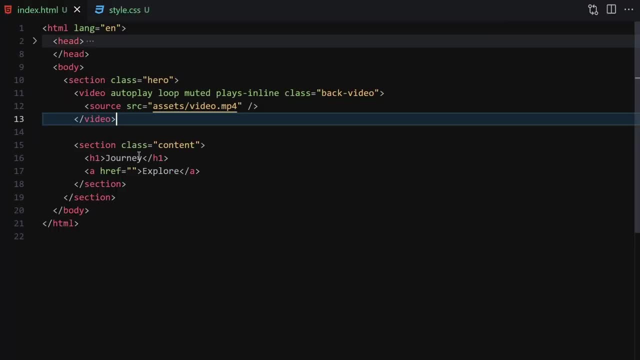 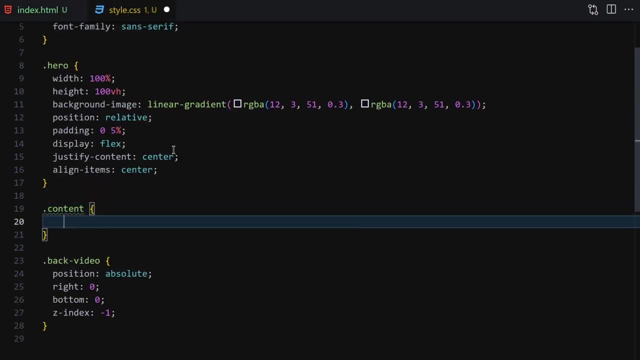 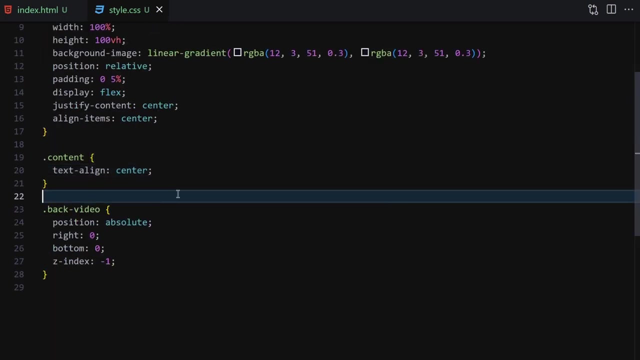 so i'll just write like: uh, select this content container. so i'll just select that, so just write like content, content. and then here i'll just write like text: align of center. and once we set our file, so everything is now perfectly center, okay. so the next thing i'll do is i'll select this: uh, h1, which. 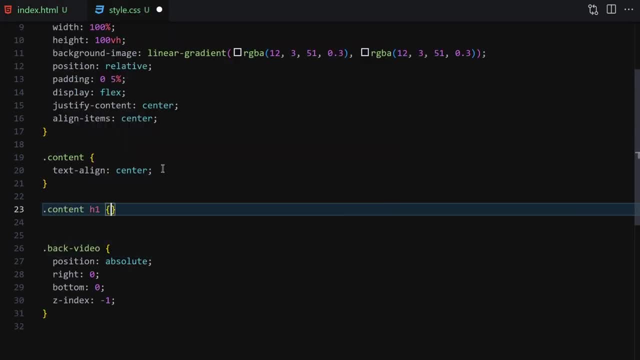 is inside this content right here. so i'll just select this content and then h1, uh, and then i'll just provide, like font size of 160, pixel color- that'll be totally white, and font where it will be 600, and then you know what? yeah, i guess font where will be 600, and then i'll just provide a transition. 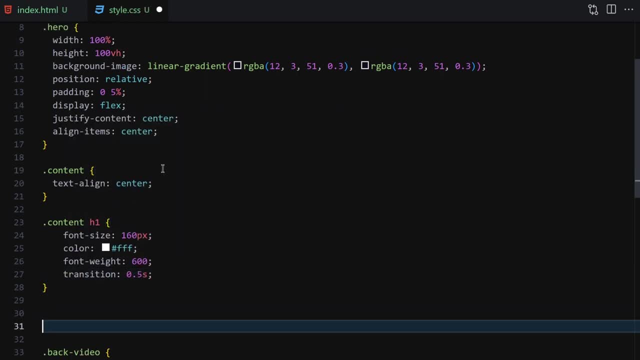 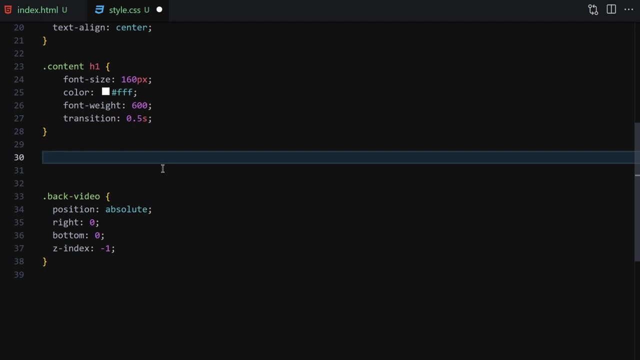 of 0.5 second because i want to provide a hover effect to it. so that's why i'm writing a transition and it will take five seconds and 0.5 seconds to be precise, not even one second- and then i'll just select this content and then h1, and once we have over that, h1. 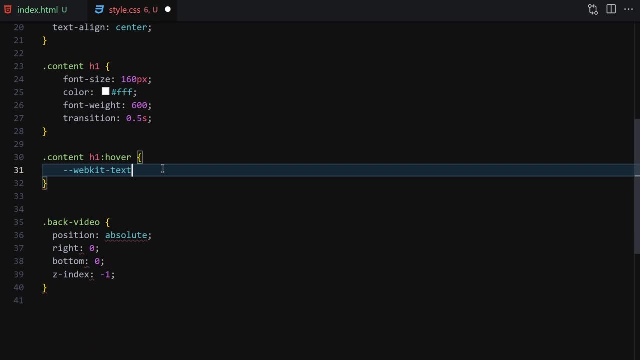 so we want to provide, like web kit dash text, just one uh dash, not dash, dash, dash, and then i'll just provide this content and then h1 and once we hover over then h1. so we want to provide, like web kit dash text only to one: uh dash, competition cover over, then h1 and we do. 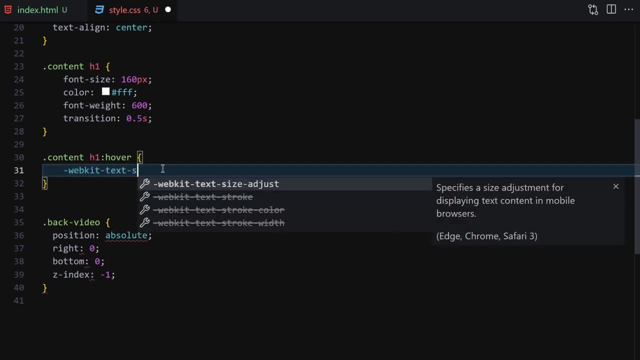 just one, uh, dash, now dash, dash, and then add one and the while keep going like: okay. besides, feel free to untited have to go smaller, like тяж amazing stuff in the out there we will write about for like text. i'll just provide like stroke and it will be: now equals to two pixel, totally white, okay, and then. 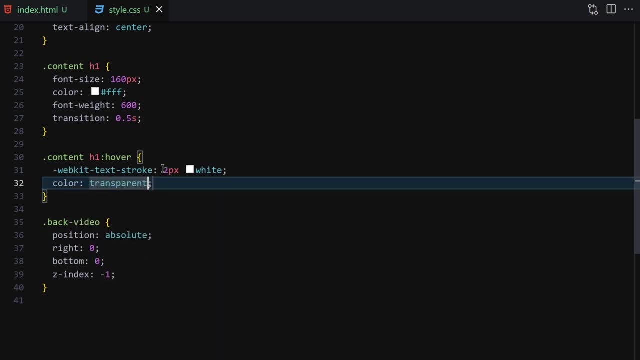 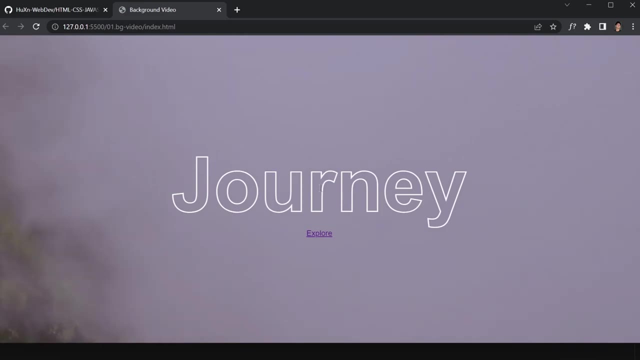 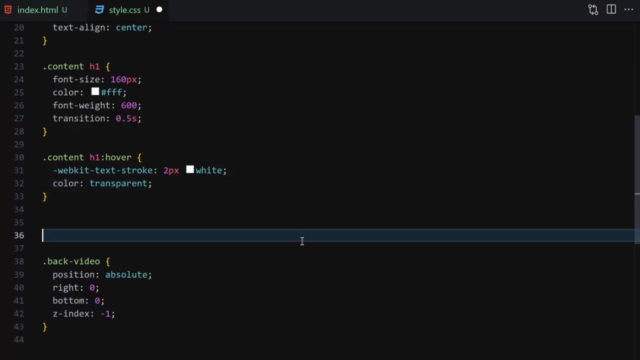 i'll provide a color of transparent. and once you save a file- okay, so here you can see- this is now our text. and once we hover over it- so here you can see- it will be now transparent and this is how it looks like. all right, so now the next thing that you have to style is this explore button, so i'll 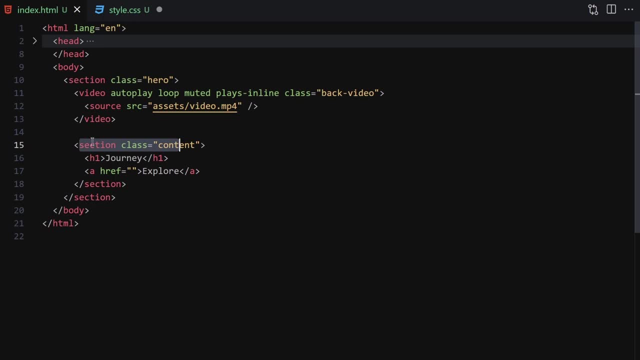 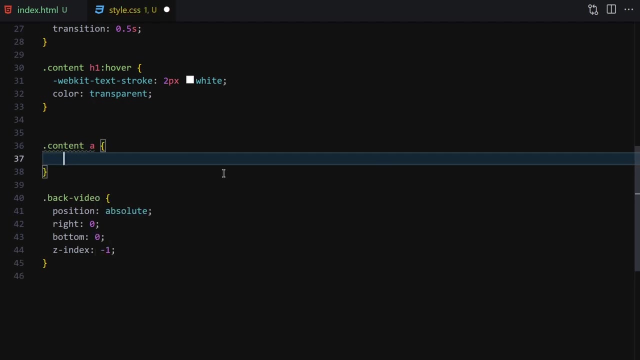 select this anchor tag which is inside this content section right here. so i'll just select this button right now, so i'll just write like content and then anchor tag. okay, inside this anchor tag i'll just first of all remove that text: decoration of none. so here you can see that decoration is gone. 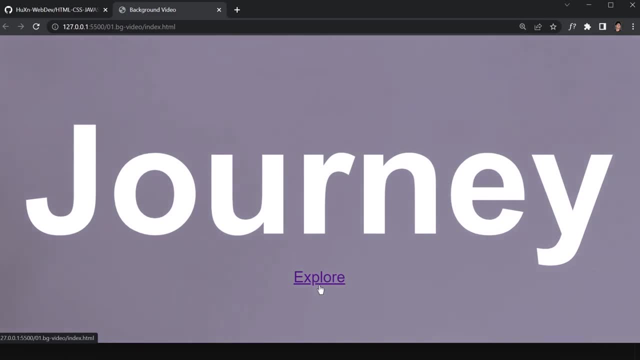 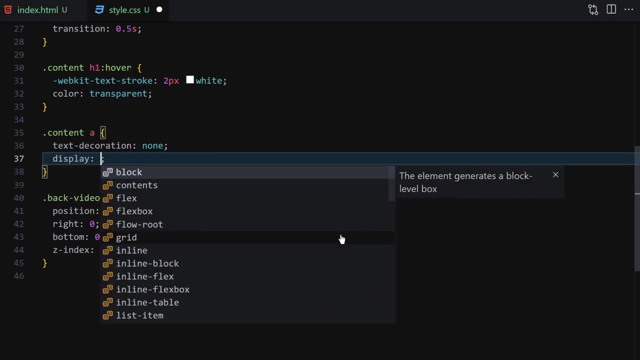 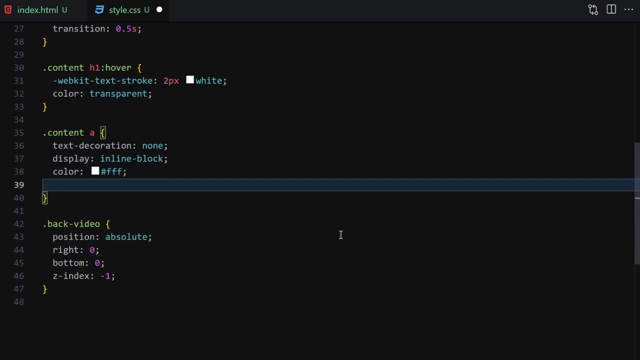 so once i uncomment it, so here you can see, we have this decoration right here like underlying decoration, and once we uh, remove there, so here you can see, that's removed. display of inline block, and then i'll just write a color of totally white and font size. 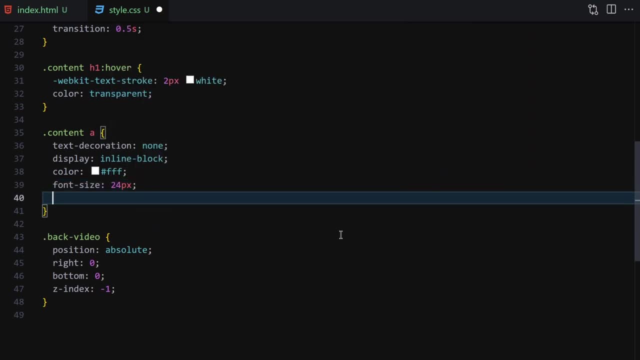 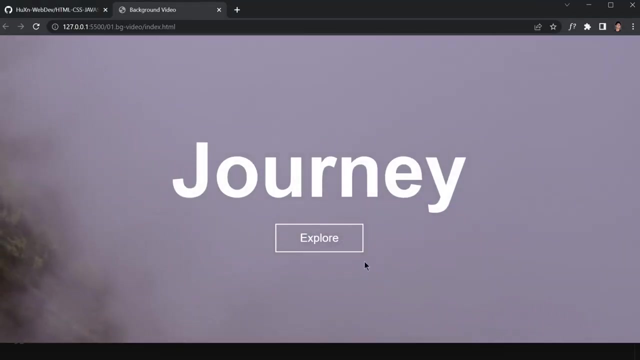 will be 24 pixel. by default will be 16, so now we change it to 24 and border will be 2 pixels solid, wide and padding will be 14 and 50 pixel, and then margin top will be 20 pixel and once we serve files here, you can see we have this button right here. okay, i don't know why it's not hovering. 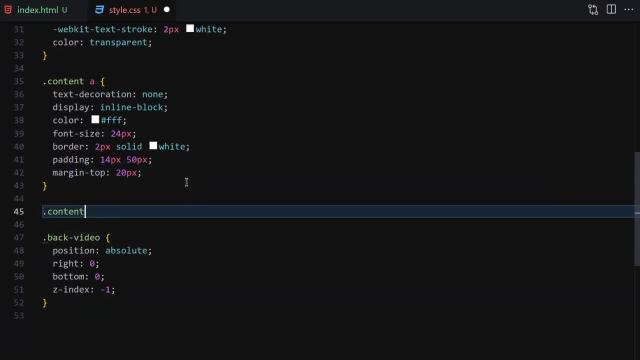 okay, we're not providing a hover effect here, so i'll just select this content and this anchor tag and once we hover over to it- so you want to provide a background color and color of totally white and the color of totally black, and once we hover over to it, so 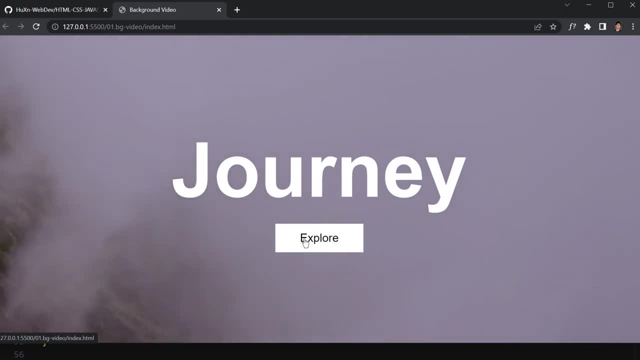 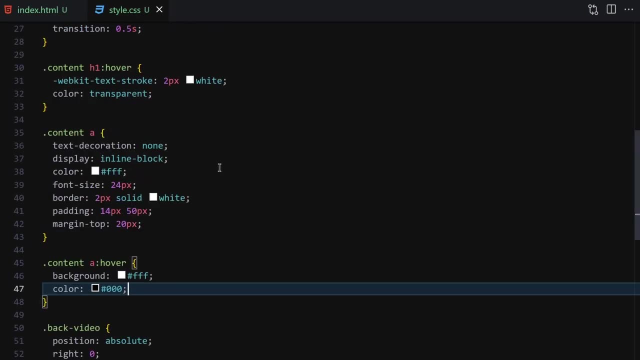 here you can see, the background is now becoming white and the text color is becoming totally black right now. okay, and it's taking one time, okay, we have to change that really quickly, i guess. uh, i have to provide a transition to here. i want to copy this transition from there. 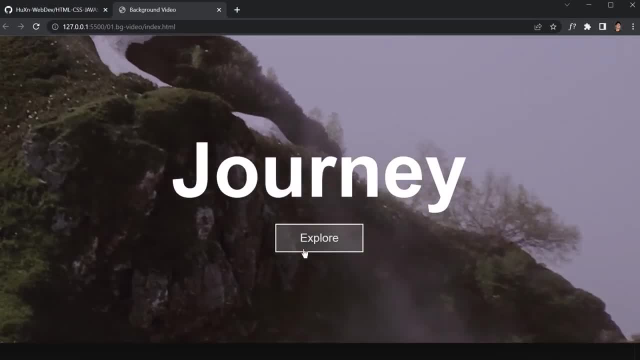 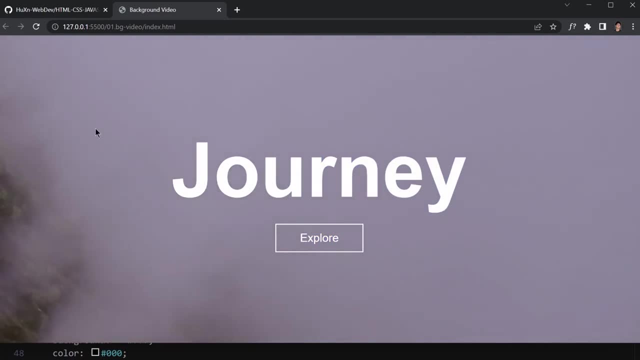 and paste it right here once we sell file and once i have my mouse ordered. so here you can see it's in 0.5 seconds. okay, so the design is complete. so now, what about the background video? now let's change the background video. so for that i'm going to have to write a media query, so i'll just write. 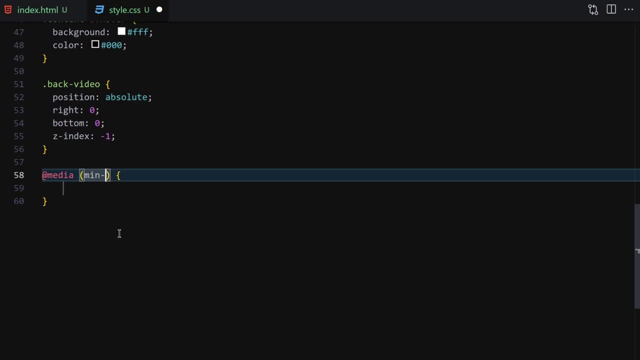 like media, and it will be just for main aspect ratio of 16 slash 9 and then we will select this back back video and then we will just provide a width of 100 percent and height of auto once we sell file. so here you can see, this is now perfectly centered and we can see already right. 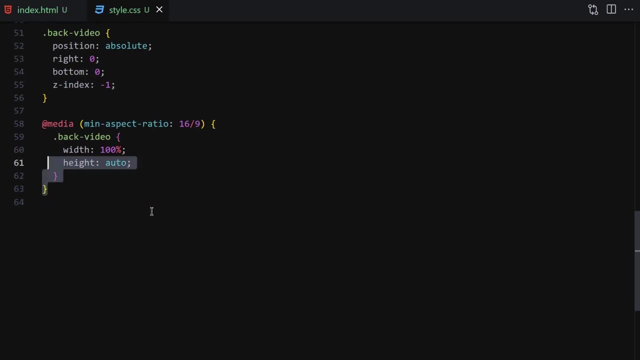 now, okay, and now let's write another media query, so i'll just duplicate this one and then change this one aspect ratio. that's correct. and then i'll just write like the first width will be auto and the height will be 100. okay, so once we set our file and then i will change this min to max. 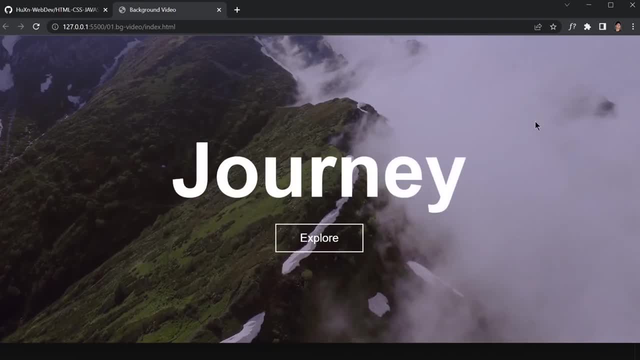 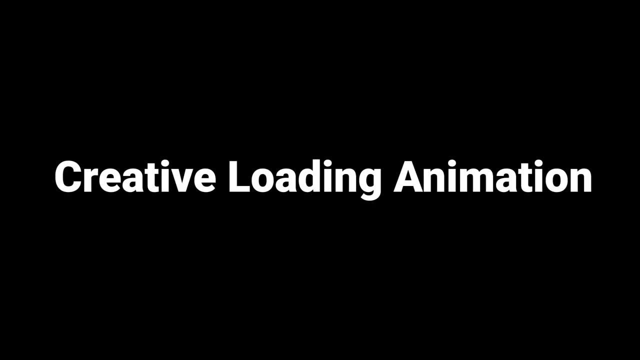 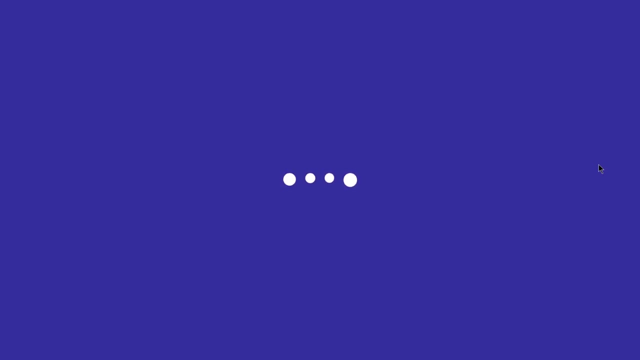 and once we set our file. so here you can see, everything is now perfectly centered and this is going to be our first project. so now we successfully create our first project in this course. hey guys, hussein, and welcome to the second project of this course. so in this video we are going to 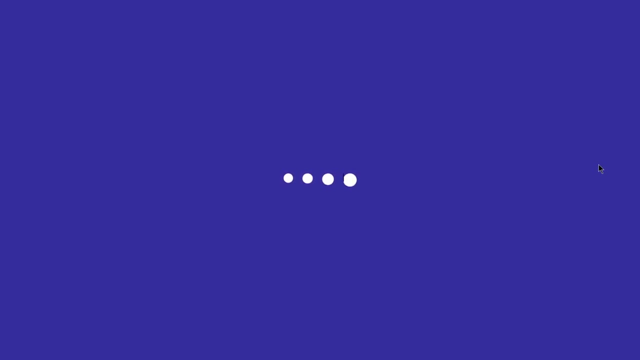 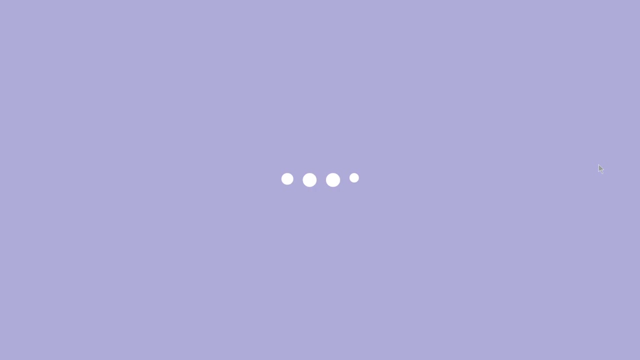 be creating this creative loading animation by just using html and css. so no javascript, no, nothing by just using html and css. so now let's jump right into our coder and write our code. in the previous video, we've created our first project. in this video, we are going to be creating 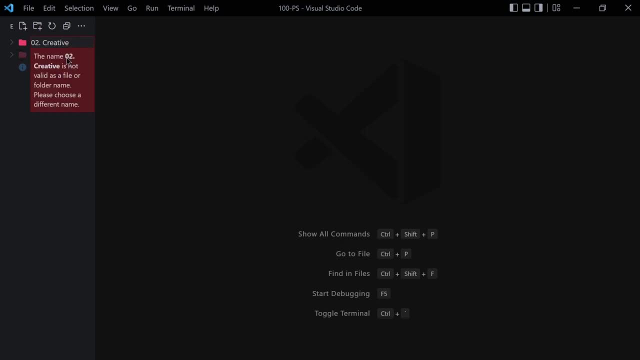 our second project, which will be creative, uh, loading animation. okay, and then inside this folder i'll just create two files given name of like indexhtml, and the second one would be stylecss. okay, so now i'll just write my doc type html very quickly. so i'll just zoom in a bit so that you guys can see everything. 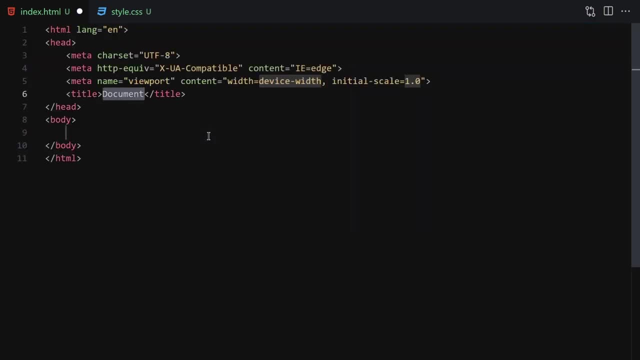 a bit better. and then i'll just write doc. and then here i'll just write like loading animation, and then i'll link it to our css file. okay, and we don't have any javascript, so we are not going to be providing any script whatsoever. and then, finally, i'll just right click on it and then click. 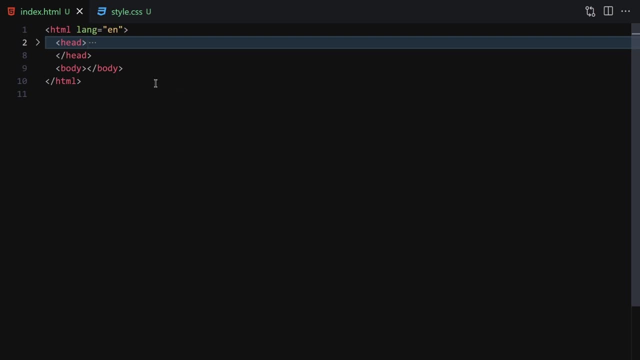 on open with the live server, so it will automatically open with, or file with, our live server. okay, all right. so here is our file right now, so in html. so we are going to be just writing a section with the class of wrapper and then inside this section we are going to have a loader. 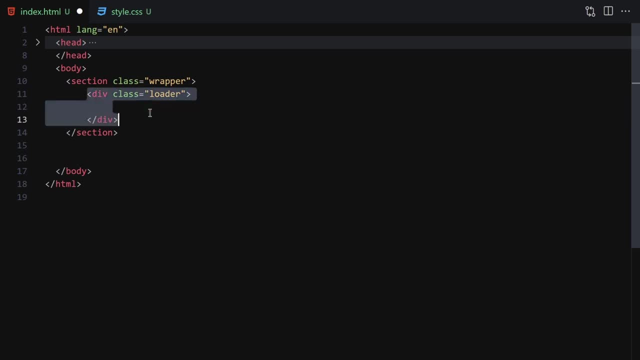 so we are going to be just writing a section with the class of wrapper and then inside this section of div, and then inside this loader. inside this loader we are going to have four um circles. so just write like loading and then i'll give a next class of one and then just duplicate it four times. 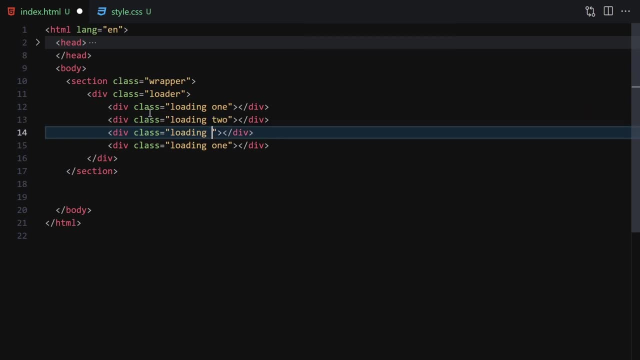 and it will be now equals to two, and this one will be now set to three and this one to four, and once you save our file, so you'll see nothing inside our browser because we didn't install anything whatsoever. okay, so the first thing we have is a section with a class of wrapper inside. 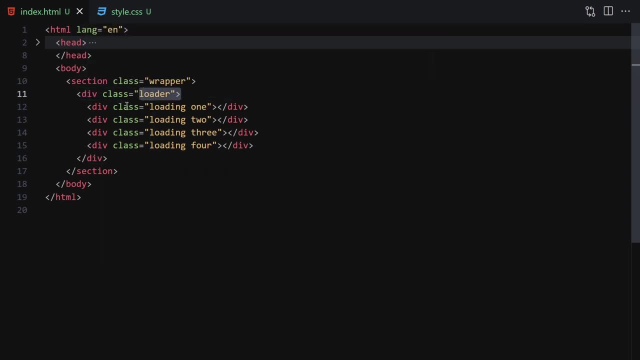 this section. we have a div with a class of loader and inside this loader class we have these four items right here and we give each of them to like loading class. we're going to style that and we're going to style specific of them, like one, two, three, four, okay, so now let's jump right into our css. so 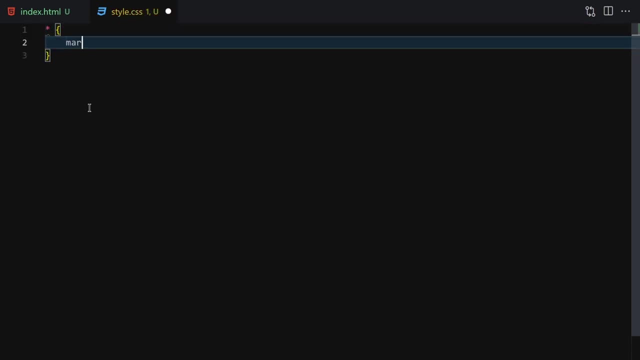 the first thing which you have to do is to just write a research for yourself, like: margin will be zero, padding will be zero and box sizing will be border box- okay. and now the next thing which you have to do is to just write a body. inside this body, we are going to be just writing a background of zero, zero, zero and one more time. 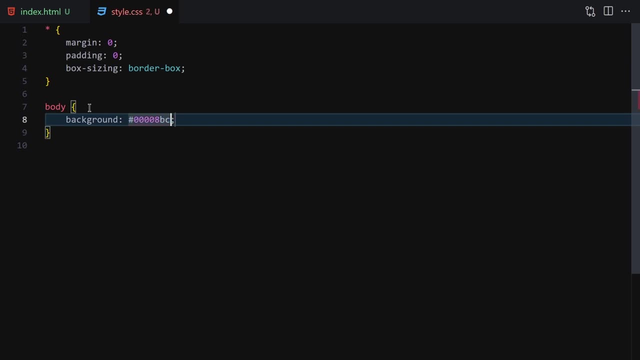 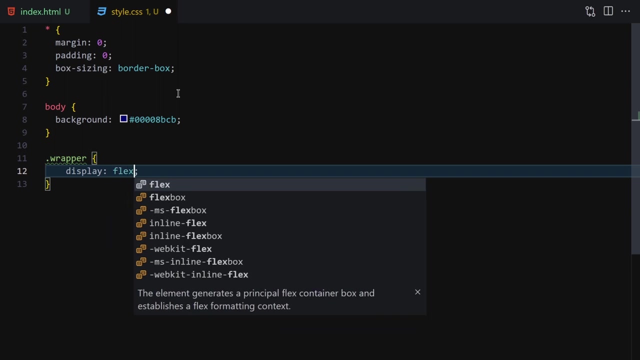 zero, like four zeros, and then i want to just write add bcb and once you save our file, so this is what blue right here. okay, so the next thing which we have to style is this wrapper section, right here. so i'll just select this wrapper and then i'll just write like a display of flags, because all 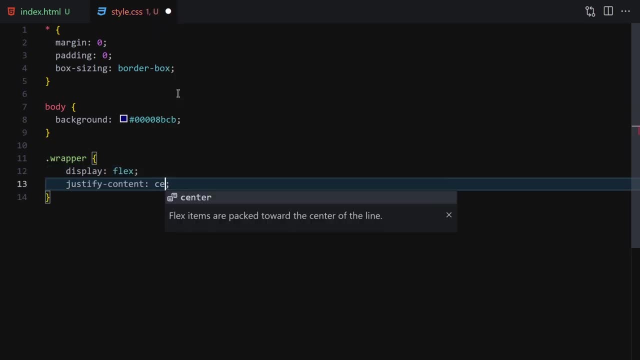 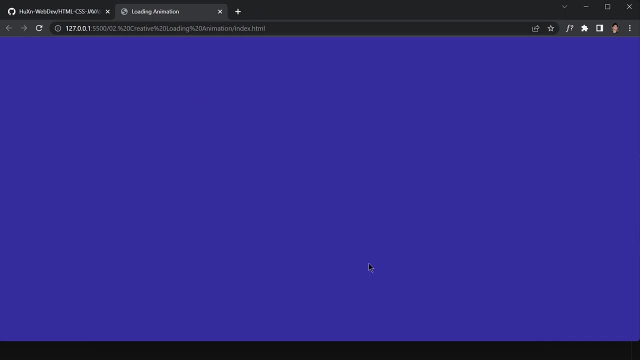 of our item will be inside that and then we are going to just perfectly center that like a line. items will be also set to center and main height will be 100 vhk. so we currently- you will not see nothing right here because we're in style or uh, loading items. if you guys don't know about flexbox, so you can check. 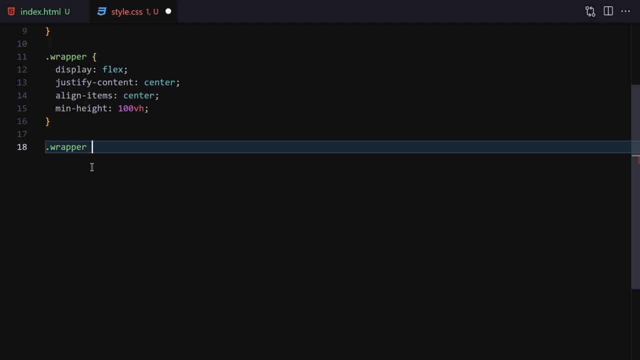 out my video on a flexbox and then i'll just write a wrapper and then i'll select this loader class right now. so just write dot loader and then inside this lower class i'll just write like: display a flex and jś charity content will be set to space between and z gy n, which should be set between: the box and just write dinner, and then we're gonna snowboard and use this image, and so that way we're gonna show you how jungs project, because you have to drag the background in the backgrounds here and we'll need to close this grain that we've just created, like as you can see, which one do you? 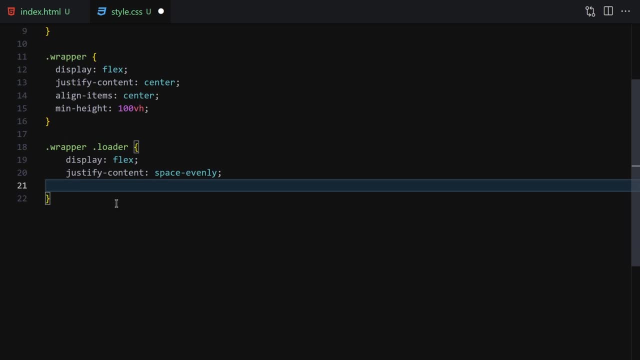 but here we go. and so then then i'm going to pass a quality content space between and then i'll just write a padding of 0 and 20 pixel, and now i want to select this loading, like each of this loading class right now. okay, so i'll just write like: um a loader. 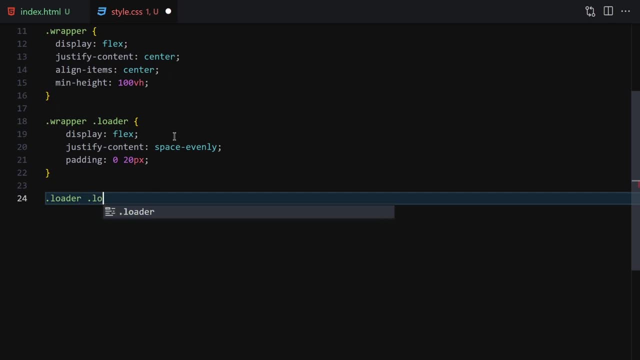 and then inside this loader, we have this loading class, like loading, okay, and then inside this loading class, i'll give a background of poorly white, like pure white, and then i'll just give a width of 30 pixel and the height will be also 30 pixel, okay, and the border radius will be 50. 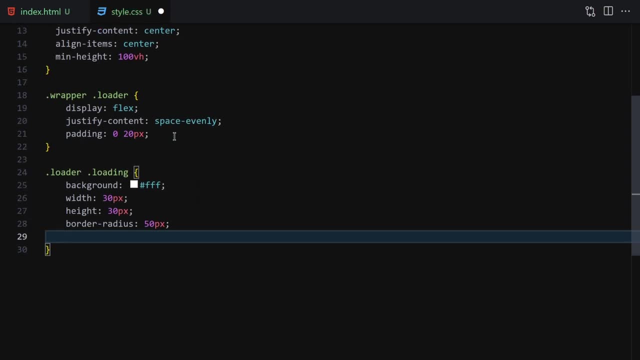 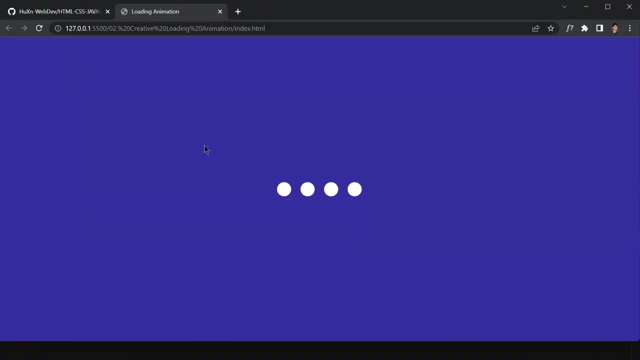 pixel, because we want them to be like perfectly. uh, circle and margin, not max resolution, but margin will be 0 and 10 pixel. and then animation: uh, we will leave there, so once we save our file. so here you can see, we have these four um circles right here and which are perfectly centered, right. 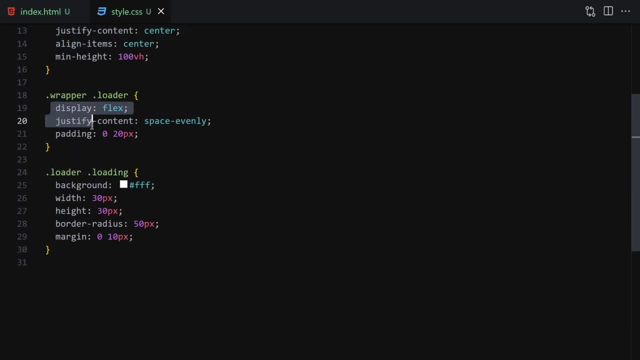 here, and here we are centering it, and here we are centering it, and here we are centering it, are just justifying it to just like, uh, to go in line, and then this class is used for each of these circles right here. okay, so the next thing i'll do is to create animation, so i'll just write like a: 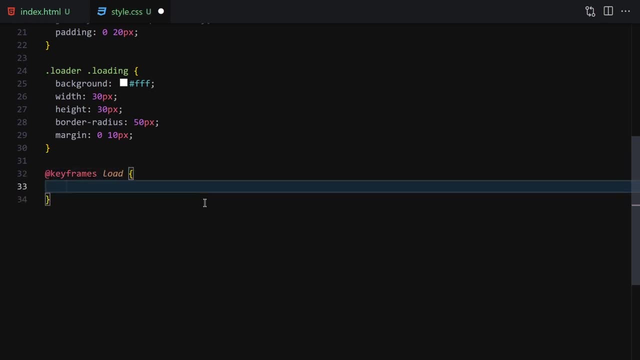 keyframe and the name will be load, and then here i'll just start from zero and then i'm going to give width of 30 pixel. i'll also give my height of 30 pixel as well. this is a starting point. when it reaches to 50 percent, then you want to just provide, like, a width of 20 pixel. 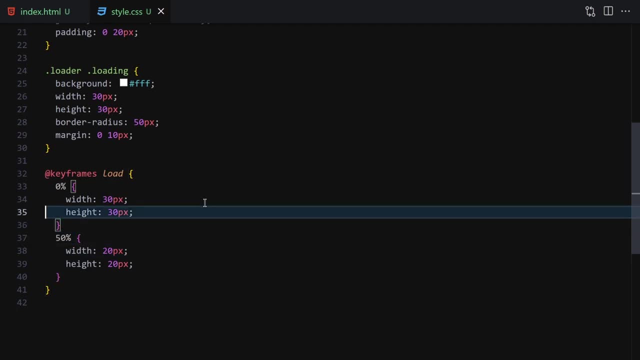 and the height will be also 20 pixels. so this is just a simple loading, right here and now. we have to provide a name of that loading animation, so i'll just write animation. okay. so it will give us a lot of properties, the name will be load, the duration will be 0.8 second and it will be ease. 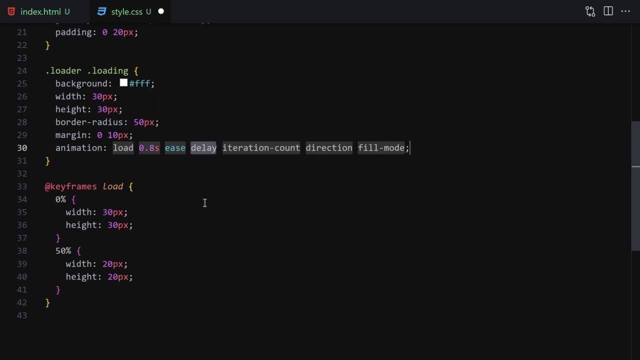 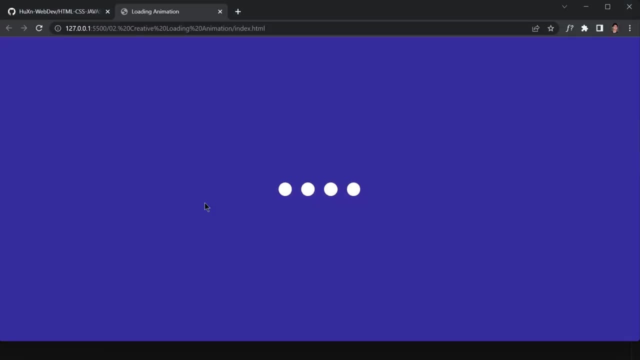 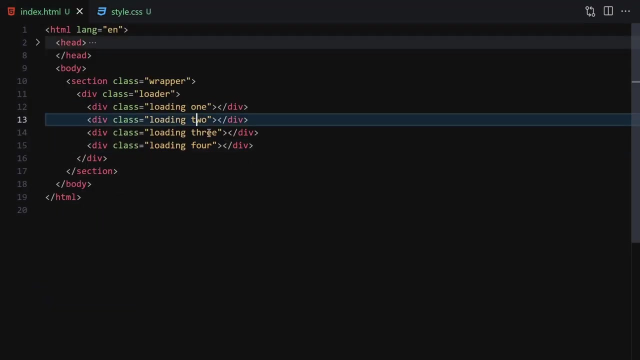 and we want them to be like delay will be infinite. so i'll just try, like in fine night and then i'll remove all of them, okay, so it will not work. it will just work like that. it will just bounce in out, okay, like zoom in and zoom out. so for that we have to select each of these classes, like one, two. 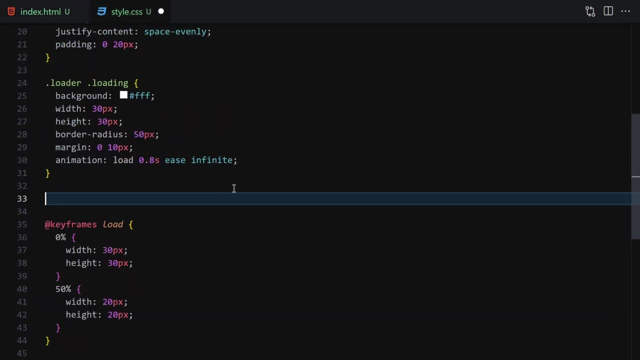 three, and we have to provide a specific animation to it, a specific delay to it- excuse my language- and then i'll just write like a loader and then i'll select my loading and then move on. okay, so you are now selecting this first one right here and we are going to 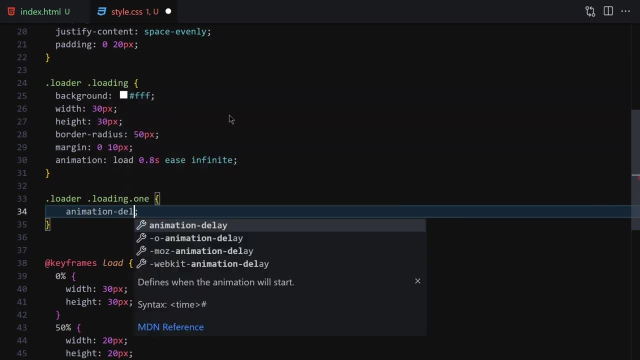 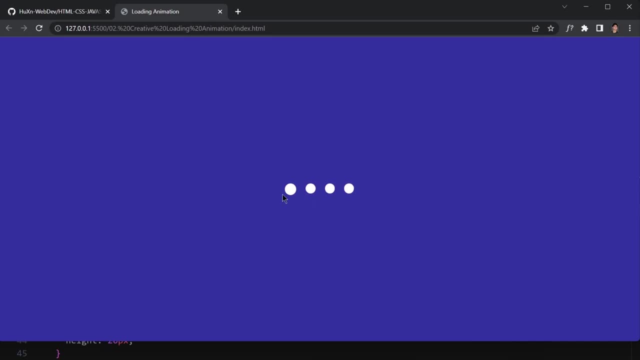 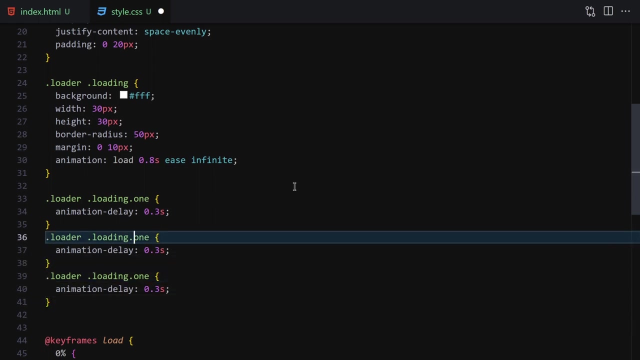 just provide, like animation, delay, not duration, but delay of 0.3 seconds, three seconds and once we set our file. so here you can see. this one is now taking a little bit of time and now let me just duplicate it four times, maybe three times, okay, and this one will be now set to. 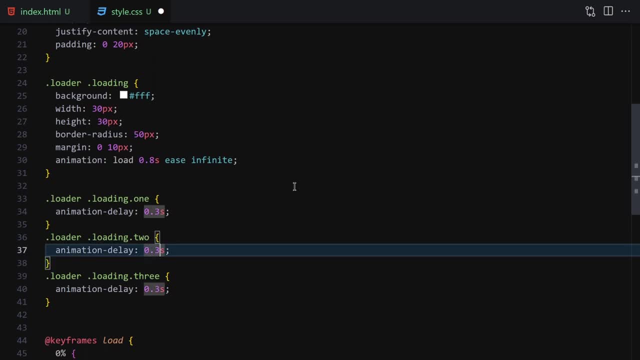 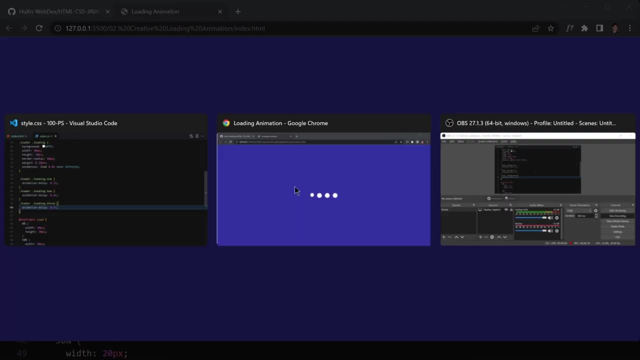 two and this one will be now set to three. okay, and now this one will be now instead of three, i'll just set that to four and this one will be set to five, and once we sell file. so here you can see, the first one will take a little bit of time and it will go on and on, okay. 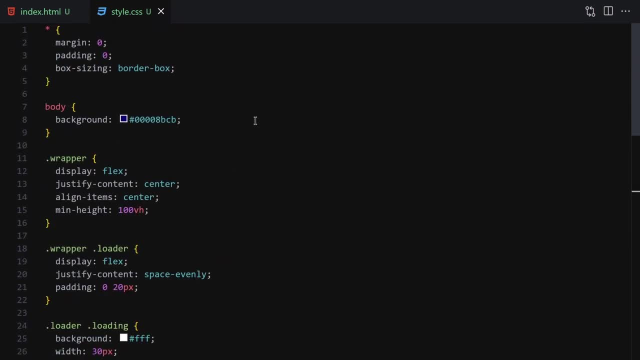 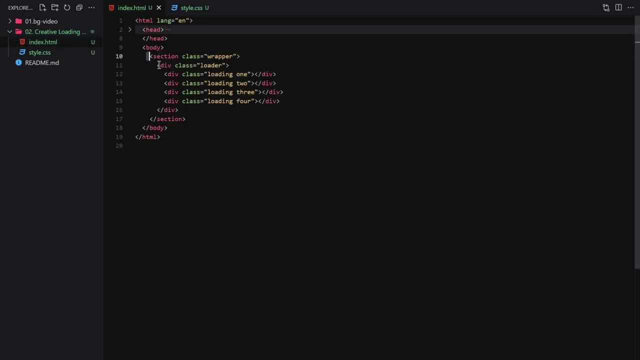 so this was our second project of this course, which is just like a simple animation, by using just html and css. so here you can see the full code. so here you can see, we have our section, then we have loaded, then we have loading items and then we just, first of 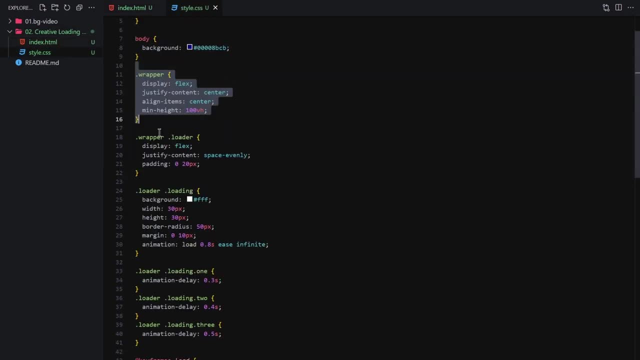 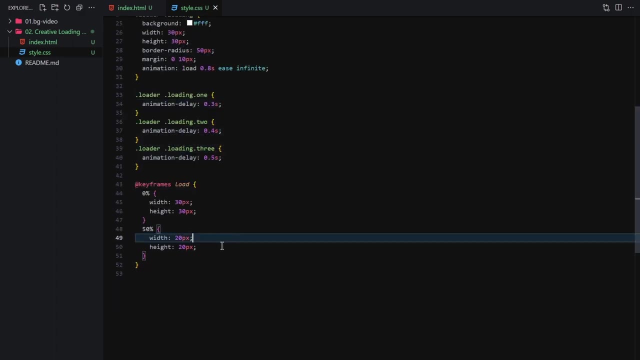 all, we have research, then we have background color and then we are scenario, then we are just uh, inlining the items and then we are providing a little bit of styling to a loading, and then we are selecting that and finally we have this animation right here. okay, 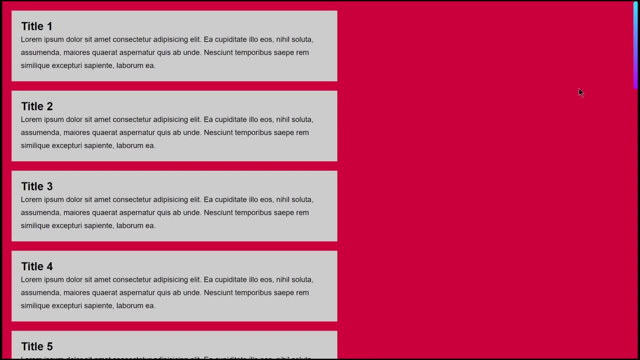 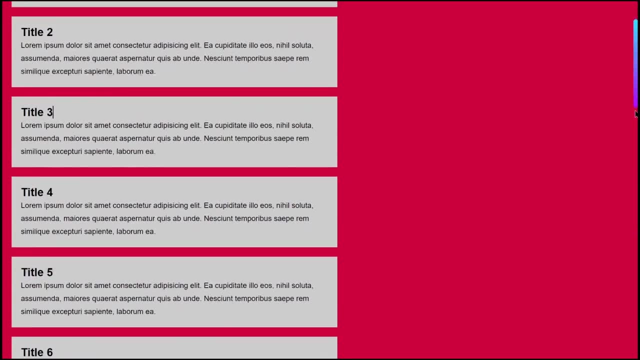 hey, girls who send, and welcome to the third project of this course. so in this video, we are going to be creating this custom scroll bar by just using html and css. so no javascript, no, nothing. so, without wasting any time, let's jump right into our code editor and write our code. in this video, we are going to be creating our third project in. 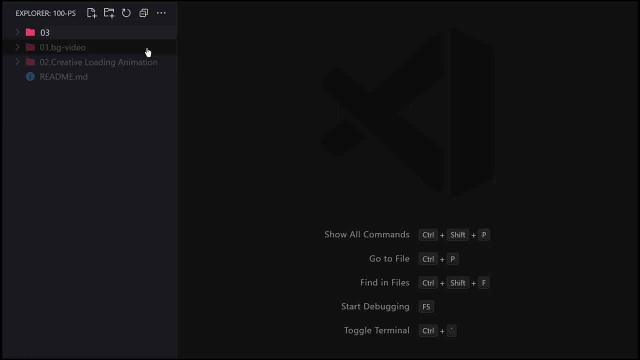 this course. so i'll just give a name of like, oh three of um, custom scroll bar, okay, and inside this folder i'll create two files given name of indexhtml and another one will be stylecss. okay, and now here i'll just write a doc type html, and then i'll go there and then i'll just type custom. 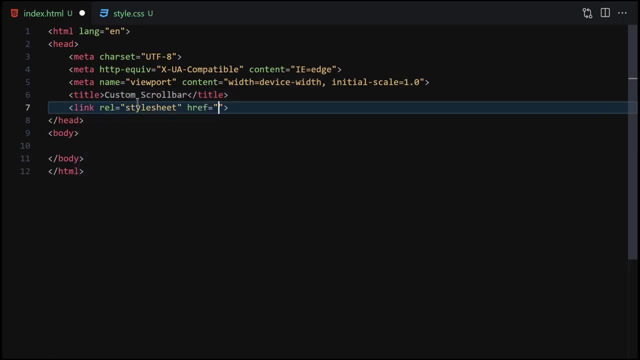 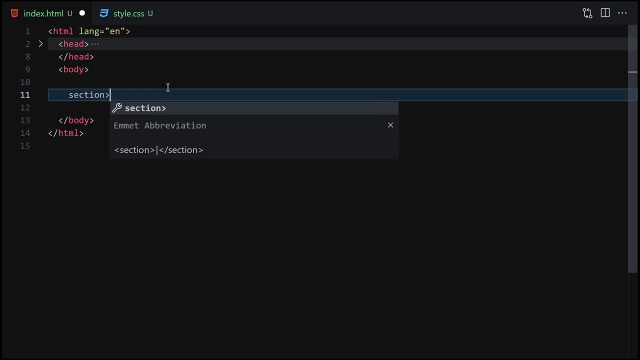 scroll bar and then i'll link it with my css file. and now we are good to go. and then i'll right click on it and then i'll launch it with live server and i'll close this metas. and now we are good to go. so for html, i'll write a simple image. so we have like a section inside the section. we 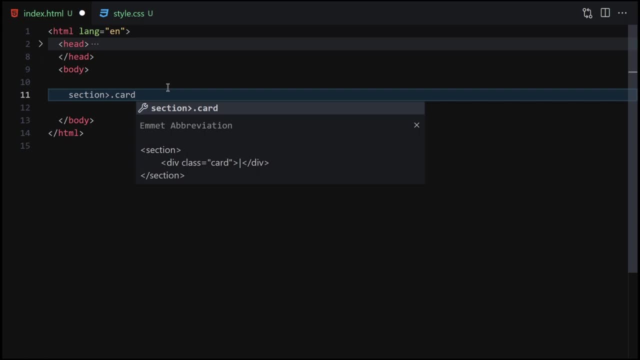 have, or inside the section we have, water current with a serpents. and outside the section we have- Oh, the card are and that's where it will show you that this script is. and inside of this section we have, or inside the section we have, what a car. and inside the section we have, what an excellent corner. 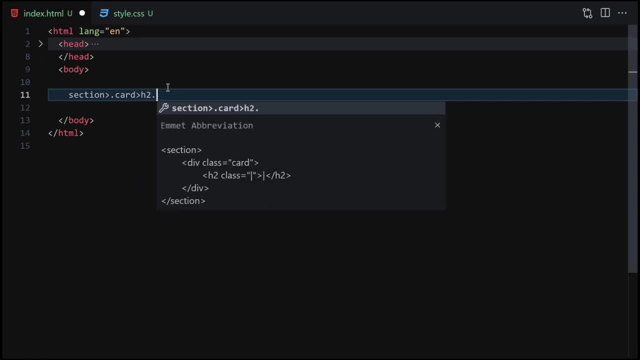 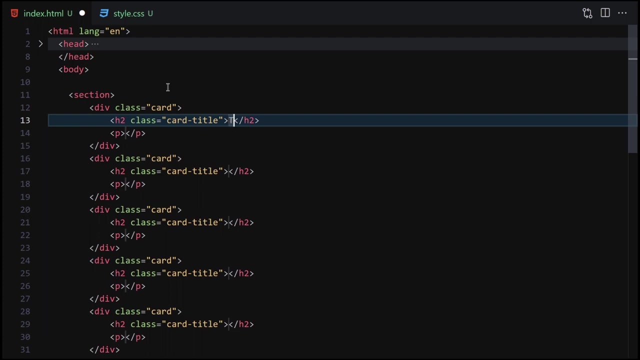 and then inside this card we have this h2 with a class of card title and then we have like plus paragraph and we want them to be eight times. okay, so remove there, and you want them to be eight times, or ten times, how many you like, and i'll just write like title one and then as a paragraph i'll 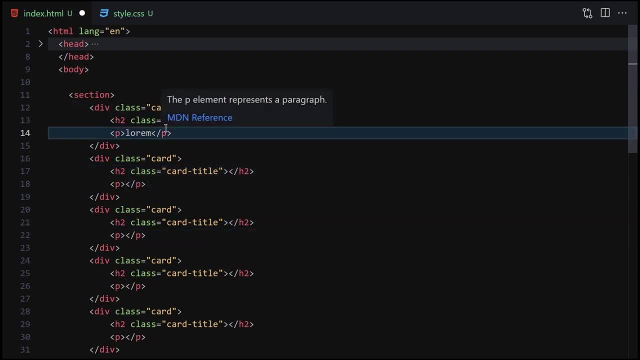 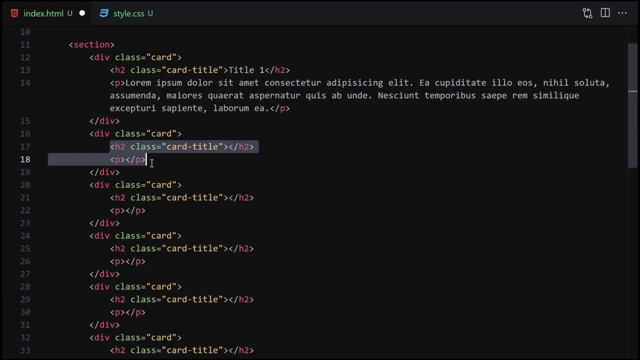 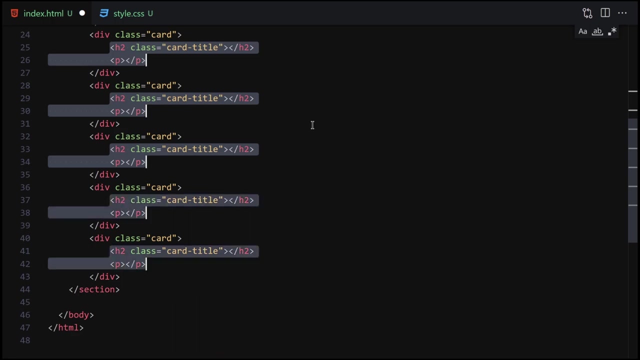 write a lorem. let me just click somewhere else and then here i'll just write like lorem, and it gives us all of that, and you know what? i'll just copy all of them and then i'll paste it right here. control. i'm going to hit ctrl d to duplicate another ctrl d, ctrl d, ctrl, d, ctrl or command d. 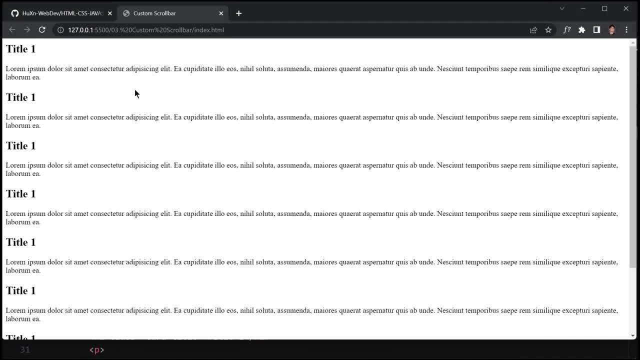 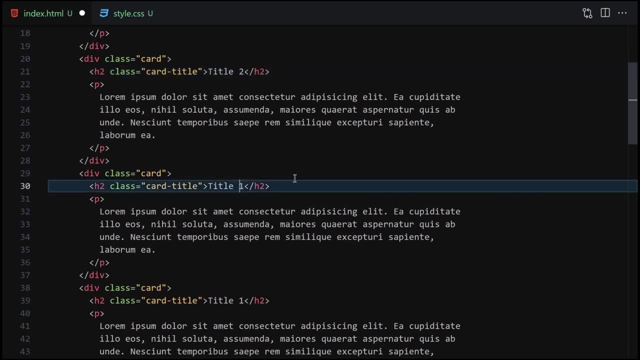 and then i'll paste all of them right here, okay, and once you save the file. so here you can see, we have this title one, title one, and all of them right now. so now i want to change the second one to two. then we have, uh, title three, then we have four, uh, five. maybe i will just 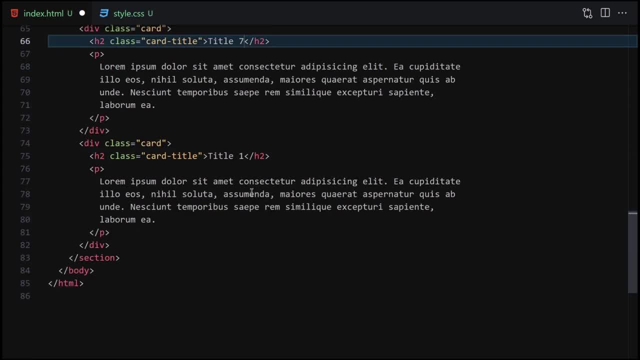 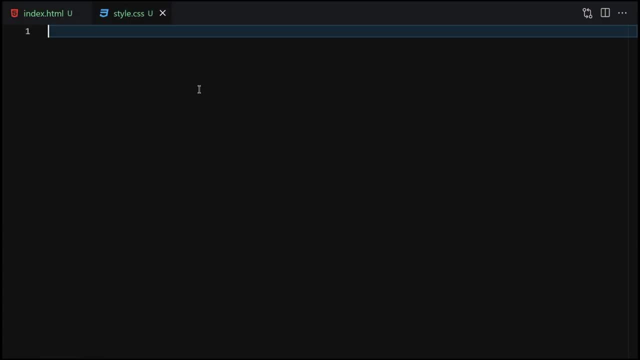 for a fast forward six, seven and finally we have a add one and once we set a file. so one, two, three, four, five, six, seven and add okay. so now let's begin with the styling. so first of all we have our resets, so i'll just provide a padding of zero and then margin will be also zero and box sizing. 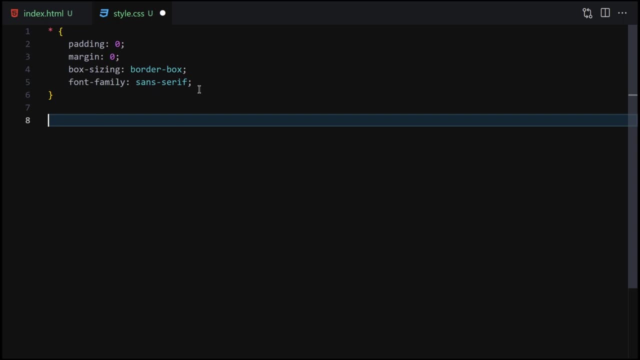 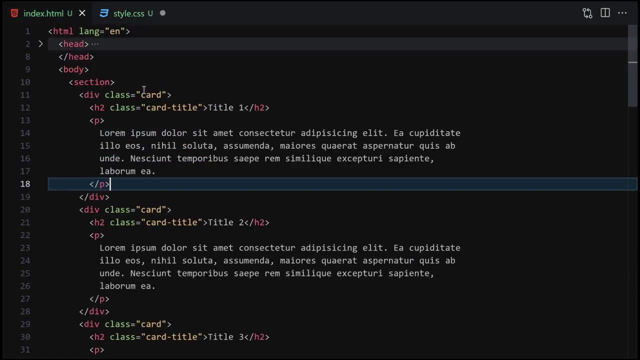 will be border box for family will be censored, and then i'll just select the body and background will be crimson and once we set a file. so here you can see it looking ugly. now we have to select this card and we have to style this card manually, so i'll just 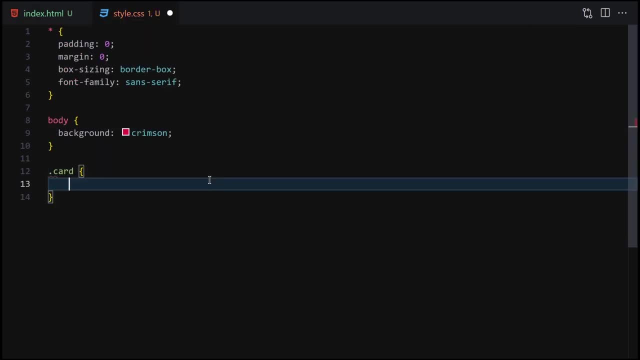 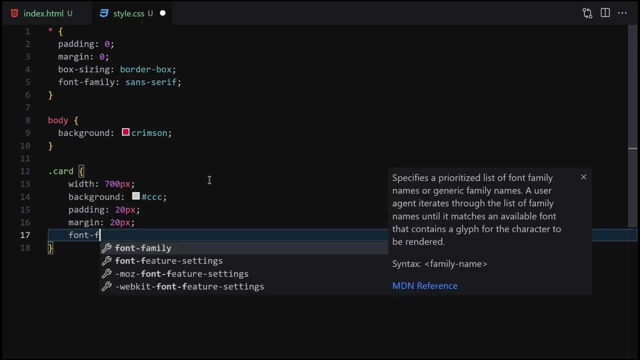 select this card and not carried but card. and inside this card i want to give a width of like 700 pixel and background will be totally ccc and padding will be 20 pixel and margin from all of them will be also 20 pixel, for family will be censored and line height i'll just provide like. 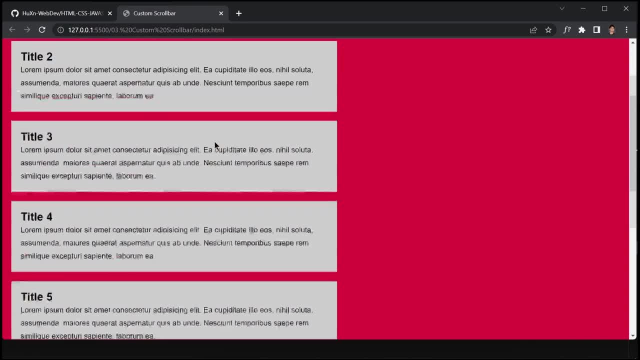 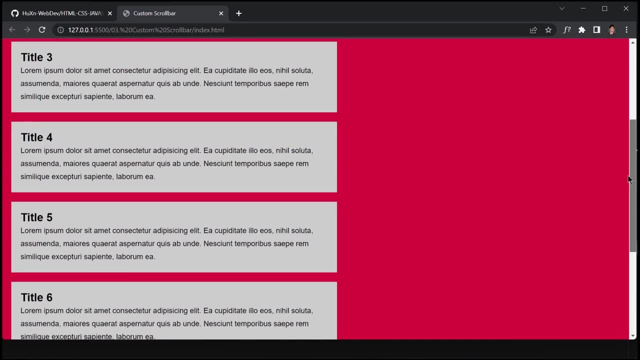 28 pixel and once we set our file. so here you can see, here are our cards right now. okay, so we have this code bar right here. the main focus of this project will be on this code bar right here, but we are just writing some text, so we have something so that we can scroll through. okay, so we are now. 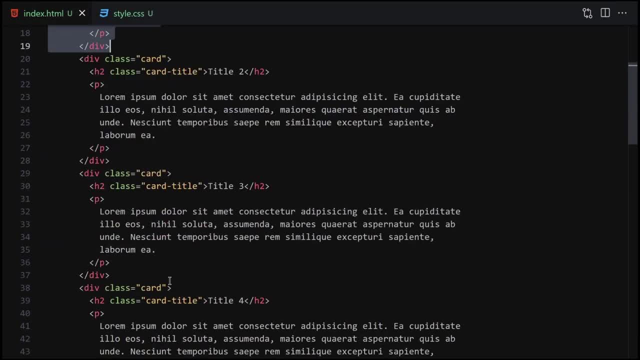 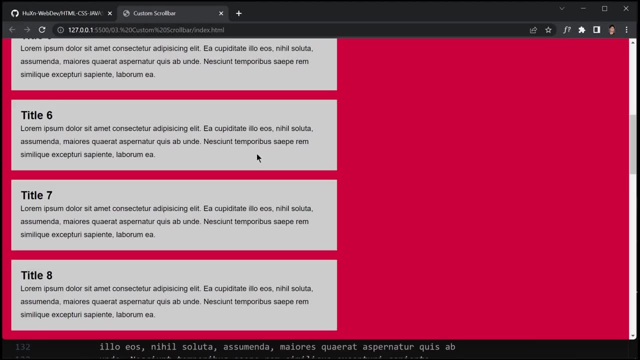 getting into like title air. maybe i will just write a few more of them. i'll just duplicate this one a few more times and we shouldn't have to change them, or yeah, i'm not changing there, but now here you can see we have a lot of. 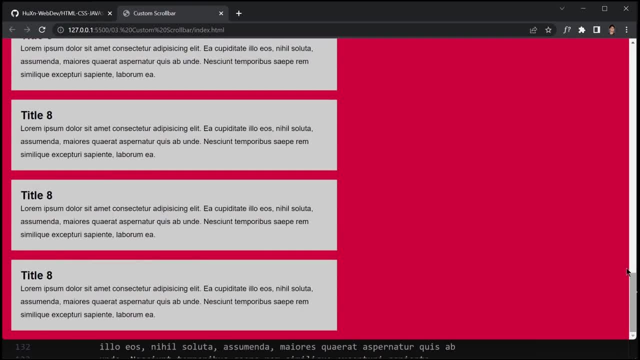 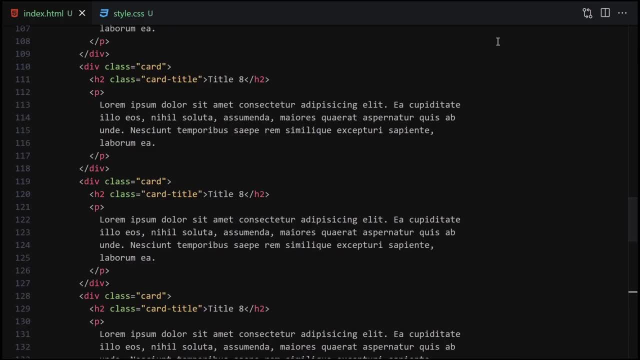 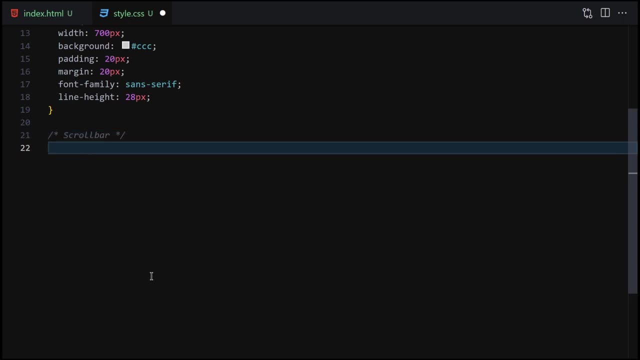 area to scroll through. so now we can focus on this scroll bar right here here. you can see that i'm talking about this scroll bar right now. okay, so how to work with that scroll bar? so for that we have to go to css. and now let's work with a scroll bar. okay, so first of all, we have to just 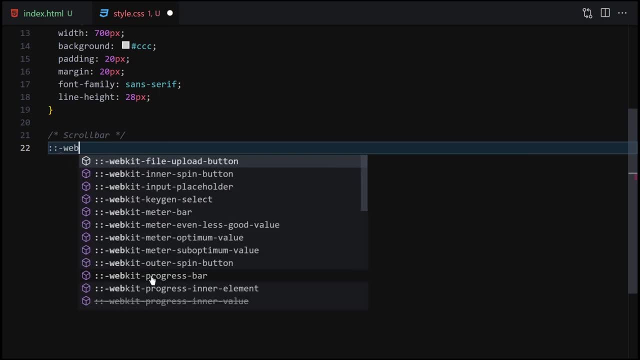 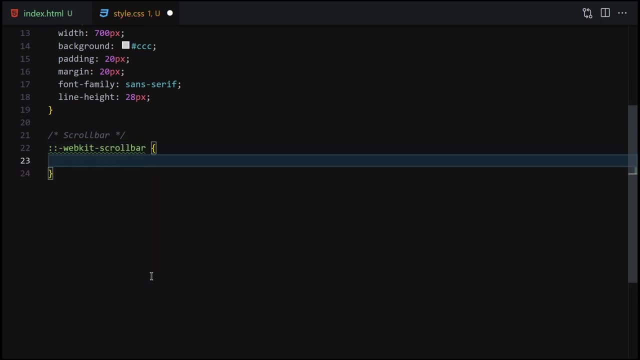 write like uh, colon, colon, and then we have to write a webkit and then dash scroll bar, okay, and so it allows us to work with that scroll bar, like, let's suppose, if i want to do like a background color to something else, like a background color to like teal maybe, and once, 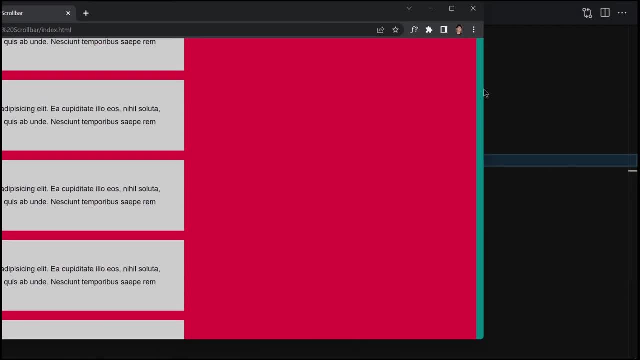 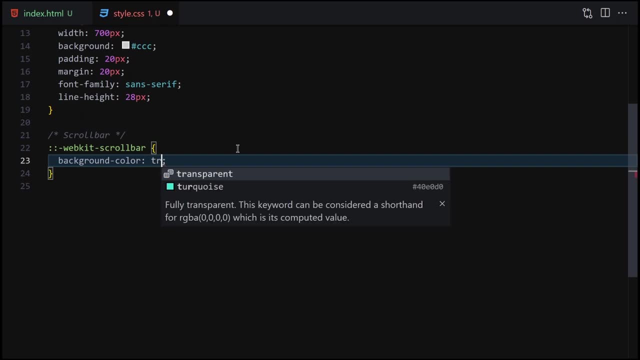 we save our file. so here you can see. their background color is now changed to teal, like all of the scroll bar color is changed to now teal, and now if you want to change that to like transparent, so i'll just write transparent and i'll just give them a width of seven. 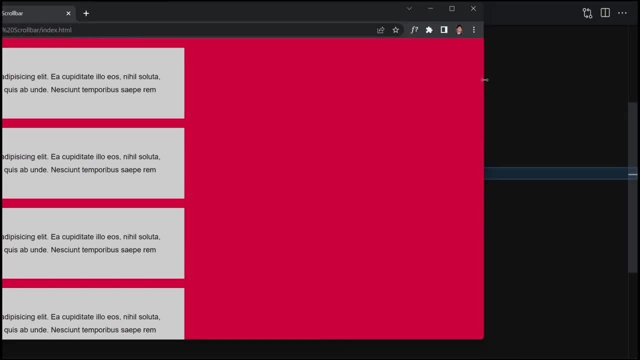 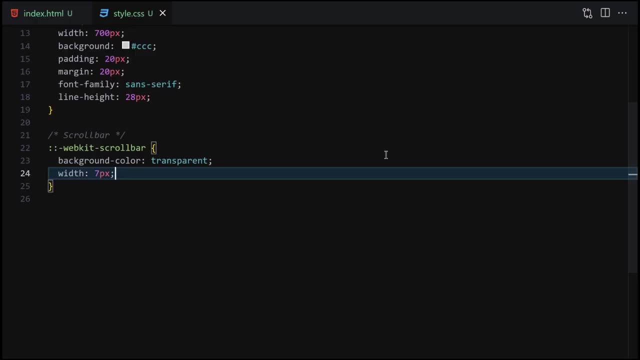 pixel and once we save our file- so here you can see- the scroll bar is totally gone because we just write the background to transparent. so now let's select the background color and then we'll select that scroll bar thumb. so for that we have to just write like: um, uh, let me just write it like: 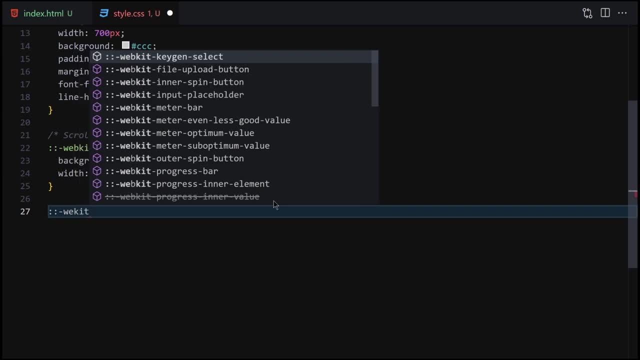 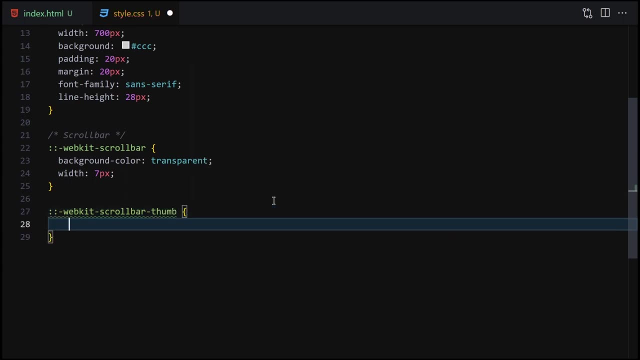 a webkit, um, webkit. then i'll just write a scroll bar and then here i'll just write a thumb. okay, so it allows us to access that thumb. so i'll just write, like a background color of, uh, i don't know, black will be fine. and once we save our file- so here you can see- it will now gives us this: 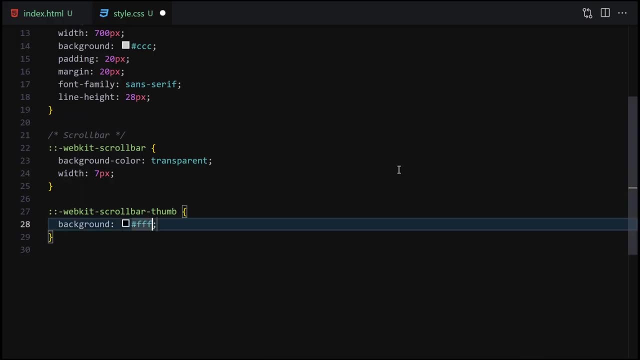 black scroll bar and if i want to change it to something else, like totally white, save our file. so here you can see, we have this scroll bar right here. so now, let's suppose, if you want to change the width of their scroll bar, so for that we have to just write like i don't know, 20. so once we save our file, so here: 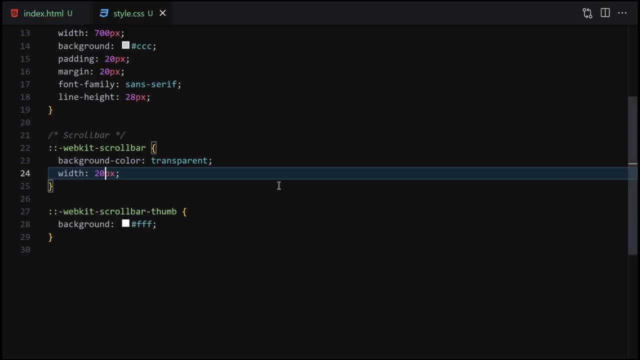 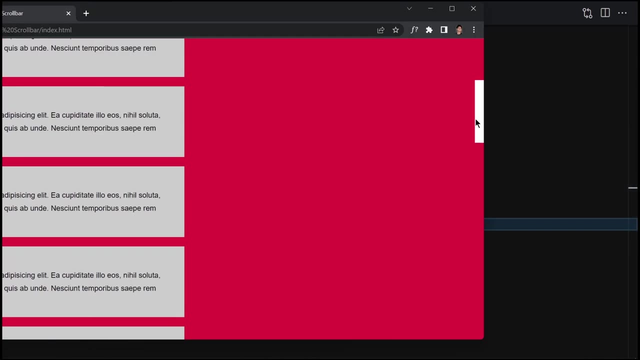 you can see, we have this massive uh scroll bar right here, okay, and so i'll just write a seven and seven will do thing. so now we want it to be like rounded, so for that we can just provide like a border radius of 100 pixels and once we save our file. so here you can see. now this is totally. 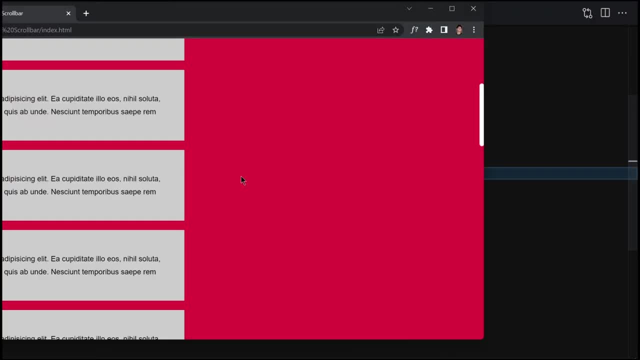 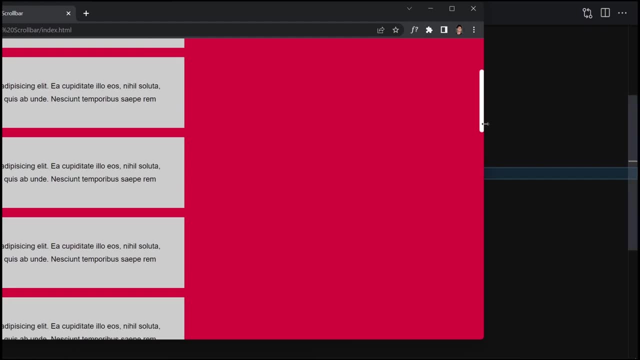 rounded. so let me change the width of it to 10.7. so here you can see. this is now totally rounded right here. so now let's suppose, if we want to provide a linear gradient to it, so we can also provide a gradient to it. so for gradient we have. 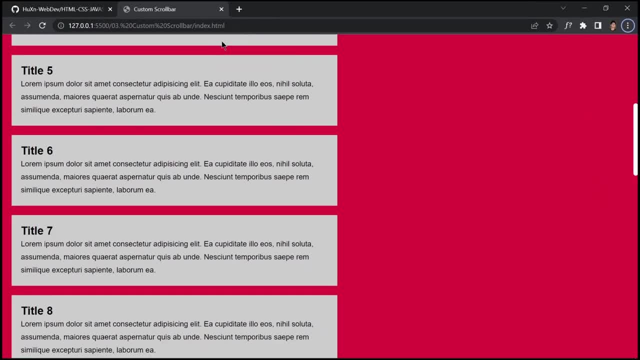 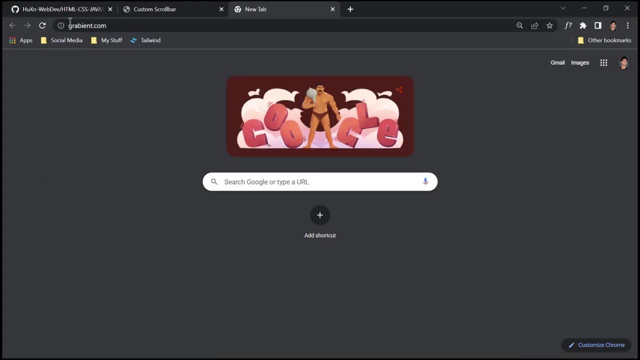 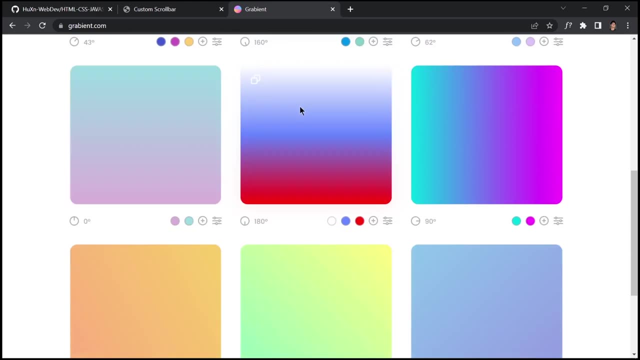 this awesome site. let me just make this screen size a bit bigger and i'll just write like gradient dot com. okay, gradient dot com, not gradient. and once we hit enter, so it will brings us to this site right here. so here we can find a lots of cool gradients right here, so i'll just click on. 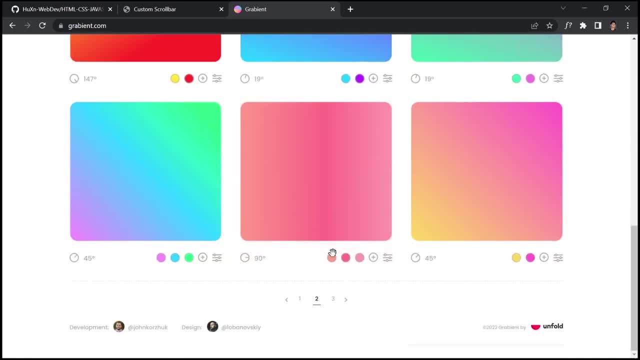 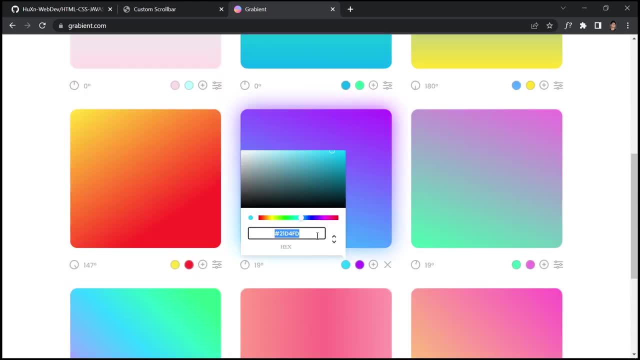 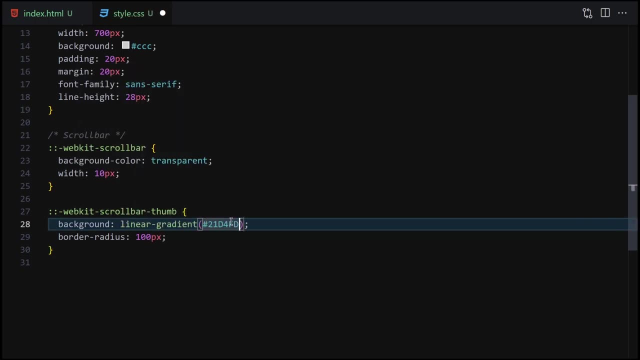 this one and let me choose a perfect gradient for myself. uh, let me see, i want to select the second one and i'll go with that one, so i'll just copy this one and instead of background i'll just write background one more time, and then i'll write a linear gradient and then i'll pass this one and 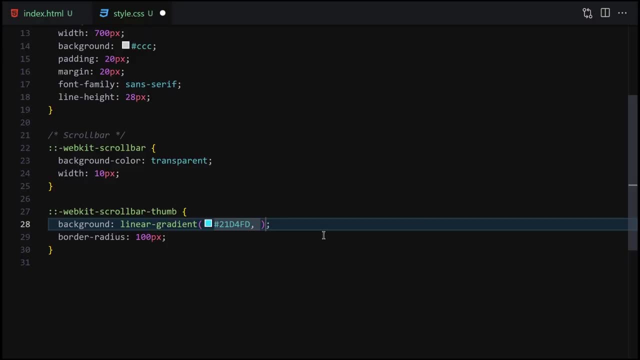 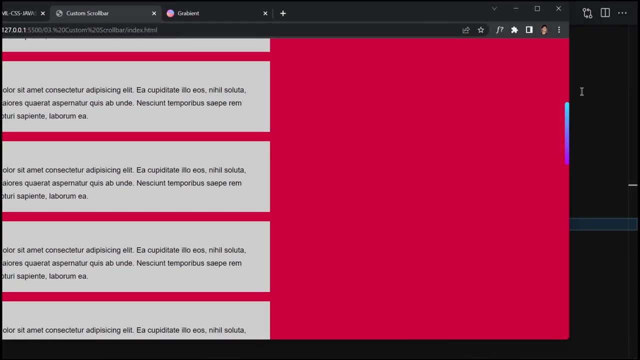 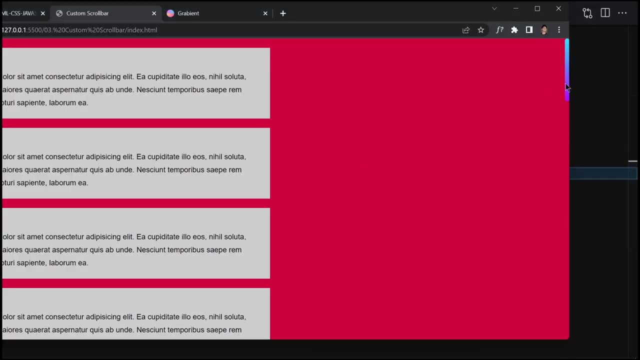 i'm going to hit comma and then copy this color, and i want to pass it one more time right here and once again. so here you can see, we have our scroll bar right here. okay, so this is how you can work with the scroll bars in html and css. so if you want to change the width of it, if you want to change the 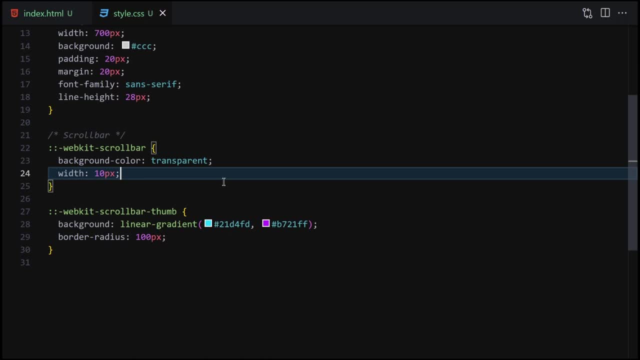 color if you want to change the style of it to something else, like maybe i don't know if i want to provide border of um two pixels, so i'm not solid, but dash white, and once we sell file. so here you can see, we can also provide a border to it right here. okay, but it's looking a bit ugly. so 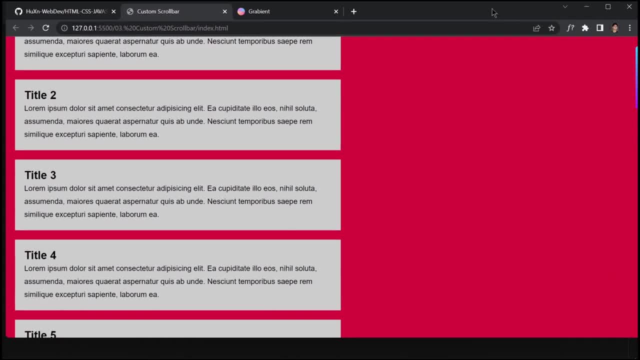 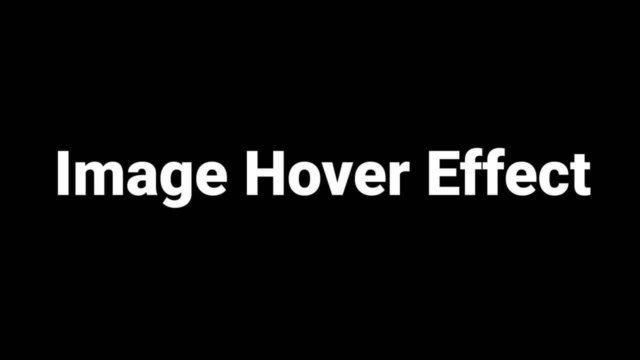 i'll just so just remove it from here. okay, so this is how we can work with the gradient. i mean, like this, how we can work with the scroll bar by using just html and css. hey guys, what's in and welcome to the fourth project of this course. so in this video, 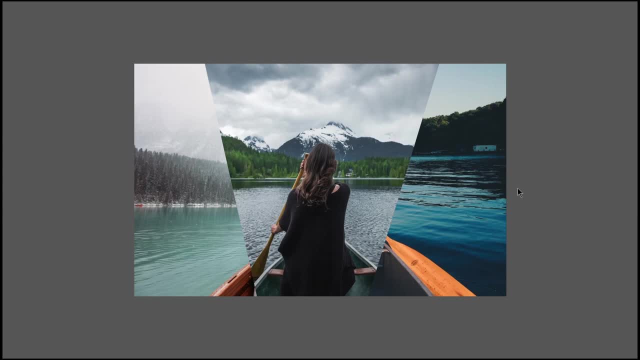 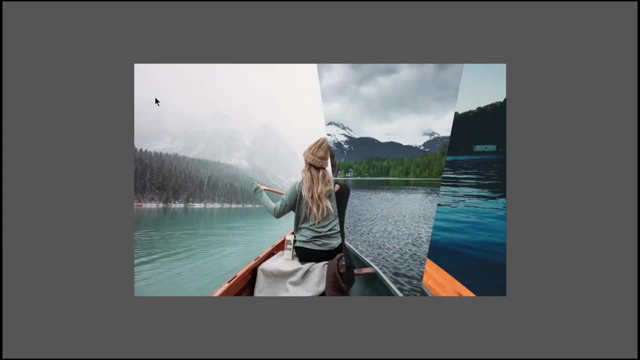 we are going to be creating this creative image effect by just using html and css. so no javascript and no libraries and no nothing. so just by pure html and css. okay, so this is what we are going to be building in this video. so, without wasting any time, let's get into it and let's get started. 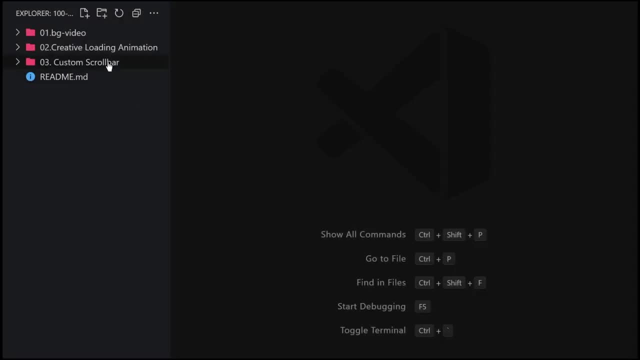 into our recorder and write our code. in the previous video, we've created this third project. in this video, we are going to be creating our fourth project, which is- what do we call it? creative image effect. yeah, i guess that would be fine. inside this folder i'm going to create two files. 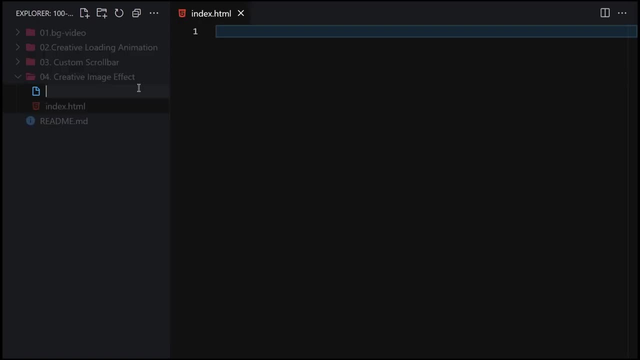 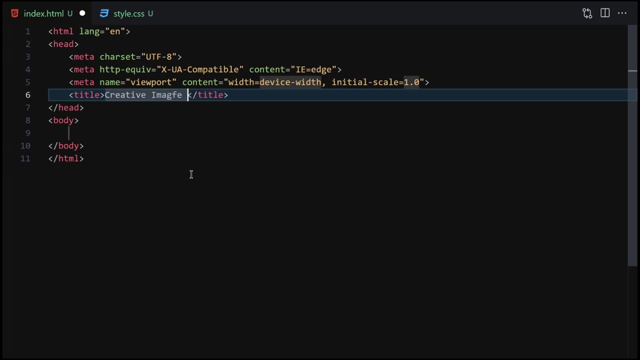 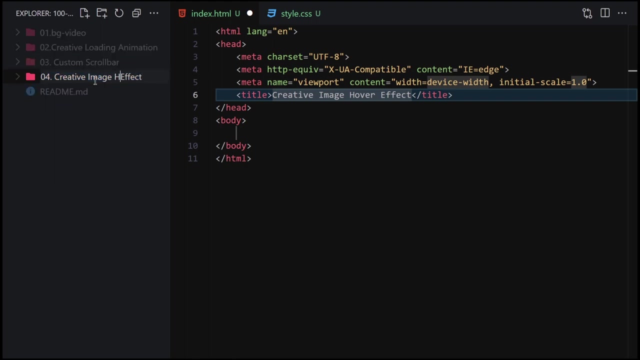 given name of indexhtml and just stylecss. okay, so now we have these two files right here inside this folder and then i'll just write like doc type: html. and then here i'll just write like: creative image- uh, how our effect? i guess i misspelled it right here. creative image, uh, our effect would. 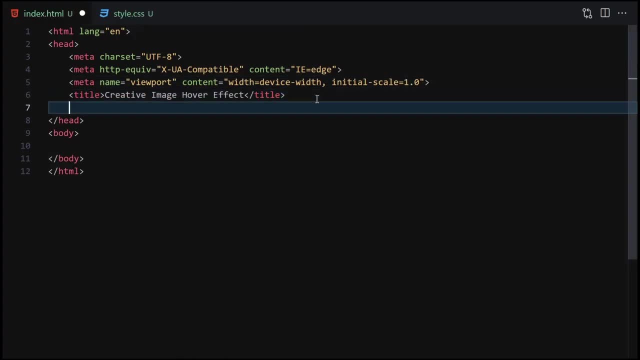 be fine instead of, uh, that just effect okay, and then we will have to link that to our css file. and now we are good to go. so now i'm going to right click on it and open with live servers. everything is working the way we expect them to work, and now i'm going to collapse. this metadata. 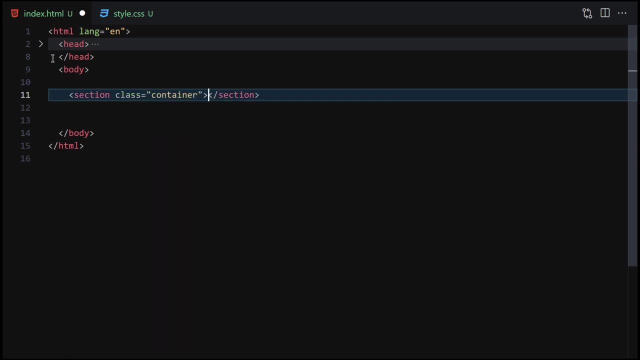 and now here i'll create a section given name of like container. inside this section we will have a few clips, so just write like clip and then clip: uh, clip one. and then i'm going to just hit tab and duplicate it three times. this one will be two and this one will be three. okay, so this is just a. 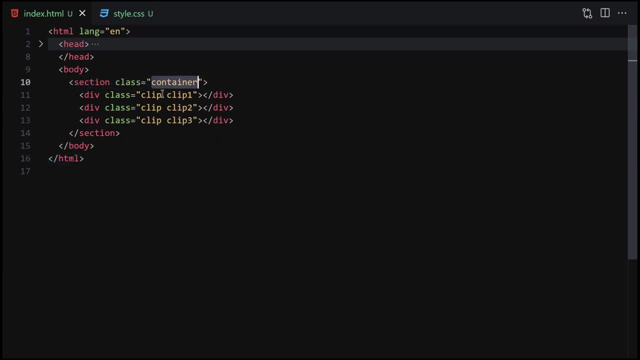 simple html right here. so we have a section with a class of container, then we have a clip class to each of these items right here, and then we have a specific class like clip one, clip two and clip three right here. okay, so this is quite simple and easy. so we're going to create a section with a 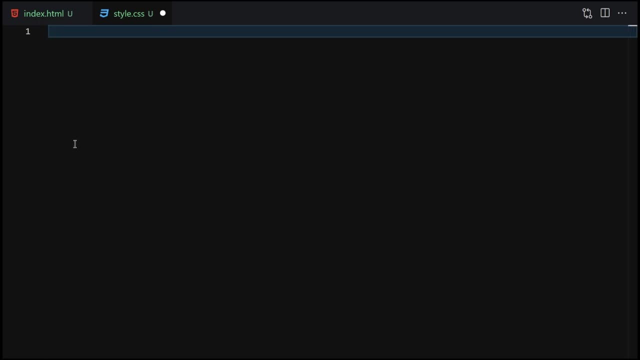 so the first thing i would do is just, uh, start from the body. so i'll just write like: body margin will be zero, padding will be also zero and background will be just five, five, five. so it will be totally gray right here, okay, so i'll also provide a height of 100 vh so that we can have 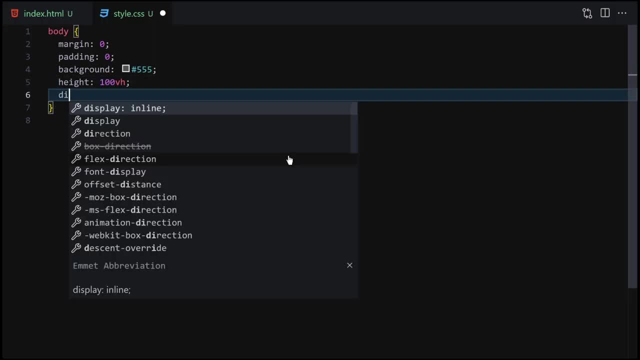 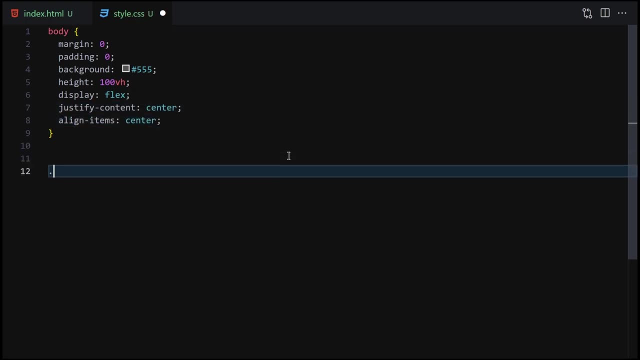 like a hundred viewport height right here, and then i'll just provide a display of flex so that we can center everything, justify content of center, align items of center, and then i'll select this container and inside this container i'll just write like a position of relative, and this width will be 800 pixel and then the height will be also not also about 500. 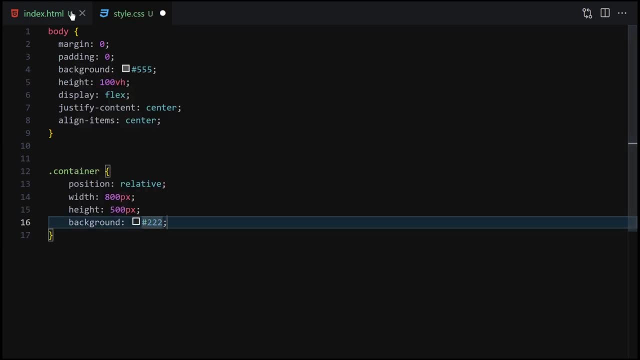 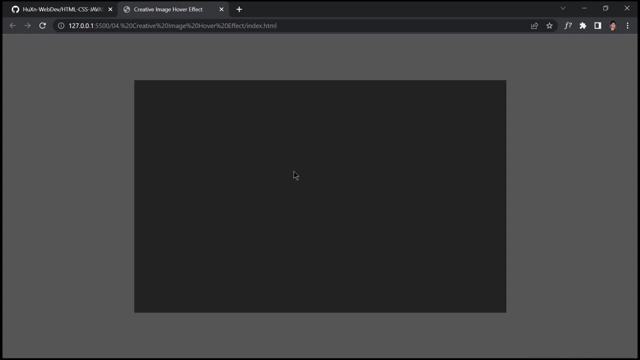 pixel and then the background will be two to two, and now we are selecting this uh container and we are just telling it right here and once we save our file. so here you can see, this is our container, right here, this is our body and this is our container inside the body. so now let's select. 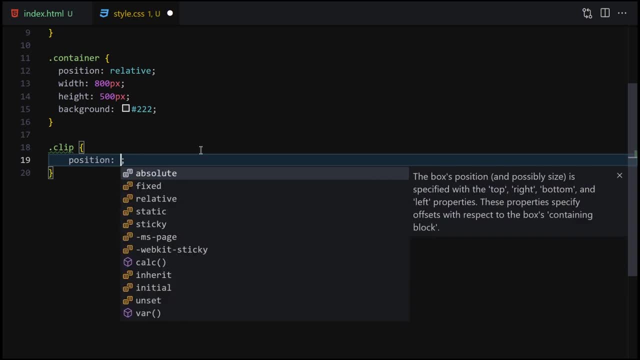 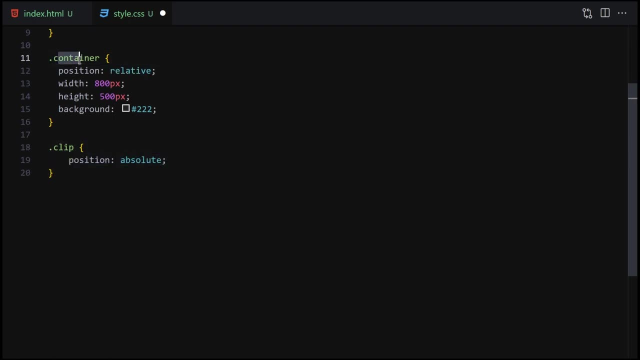 style. so i'll just write a clip and then position will be absolute. uh, absolute because this is a position relative, so we want this clip to be inside this container, so for that we are going to be writing position absolute. okay, so then we have a top will be zero and the left will be also. 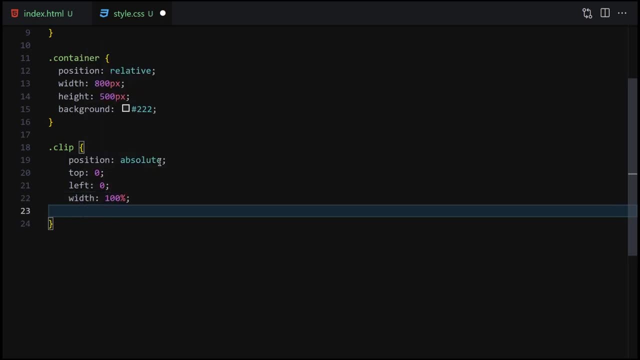 zero and the width will be 100 percent and the height will be also 100 percent. now we edge per percent, okay, and now once we save our file, so nothing will shows up because we don't have any content, we don't provide any background color. so now let me provide background color to like ccc. 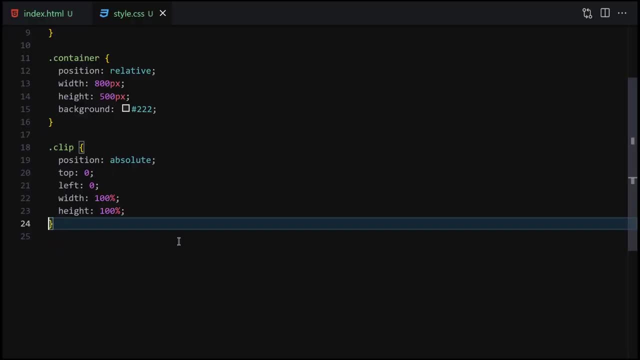 so this is our clip right here, okay, so now let's select each of the clip and then style it like clip one, clip two and clip three. so we are going to have to provide, uh, background images and we have to center those images and we also have to just clip it out, okay, so there we are going to. 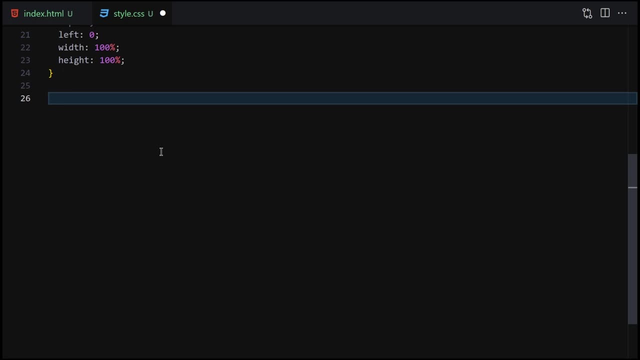 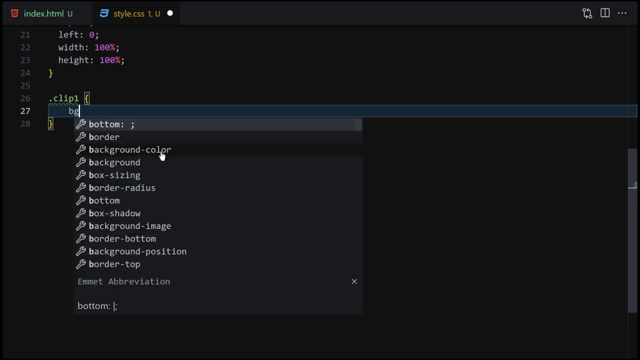 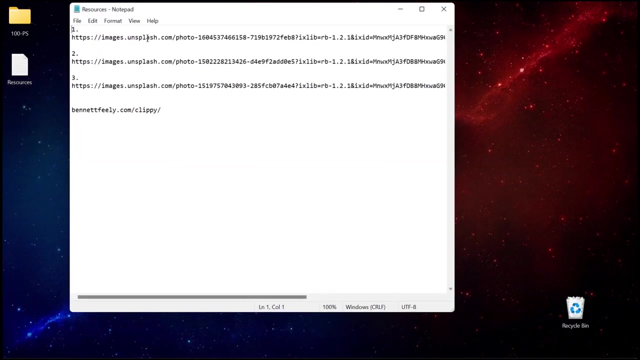 be using clip path and polygon property. okay, so now, first of all i'm going to select this clip just to clip one, and then, inside this clip one, we are going to be providing a background image, not just um, not color, but image. so here i have a few images right here so you can also. 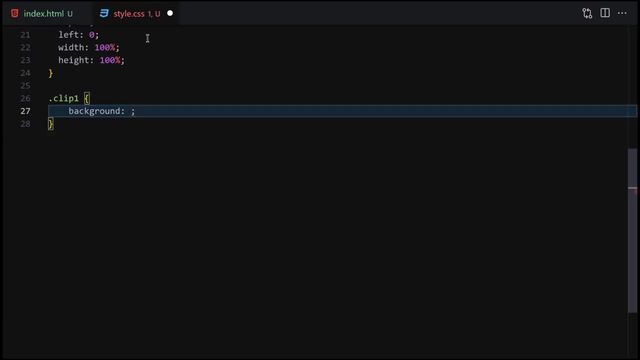 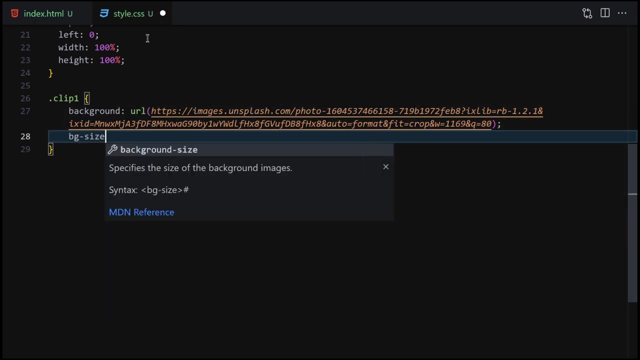 find that in the description area. i will also provide their description area and i want to paste this in the url. so this is our first image and then here i'll just write like a background size of color, okay, and then i will just write like background um position. 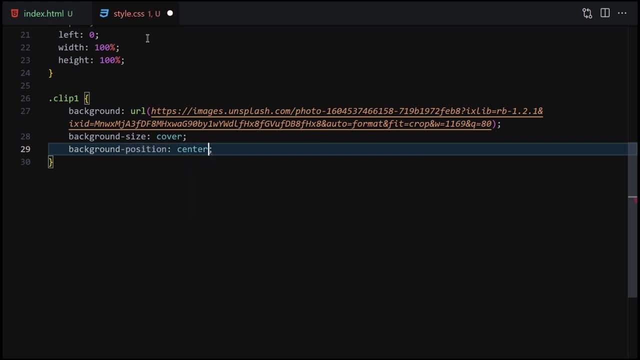 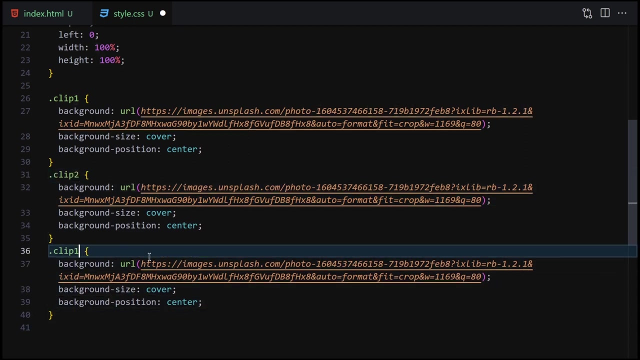 center. okay, and once we save our file, so this is our image. okay, so this is our first image. so now let's duplicate that a few times. so i'll just duplicate this one, this one, and change this one to like, uh, clip two, and this one to clip three. okay, and also, let me change the images. so again, 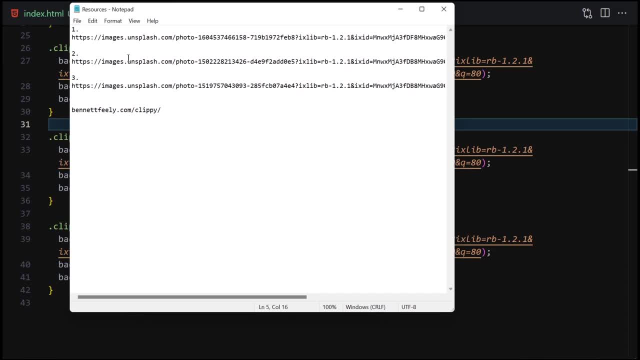 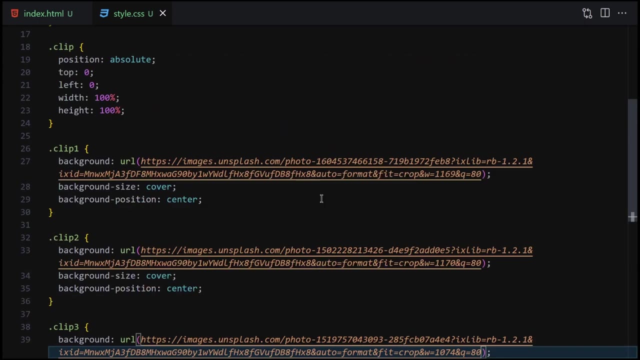 you can find these images in the description area, or you can also go to my github account, or, and you can pull that out from there as well. so this is our second image and this will be our third image. so let me copy that and let me paste that right here and the rest of them will be fine. like cover, center, center, cover. 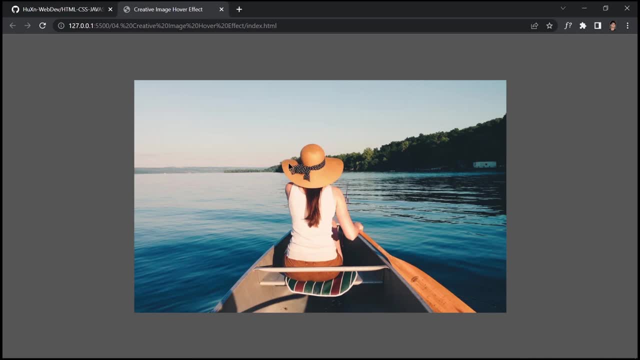 center center will be fine. okay, so here you can see, we can now see this different girl right here and this like stack at the top of each other. so now we want them to be clipped right here. so how can we clip that? so if you want to clip an image, so for that we have this website right here. 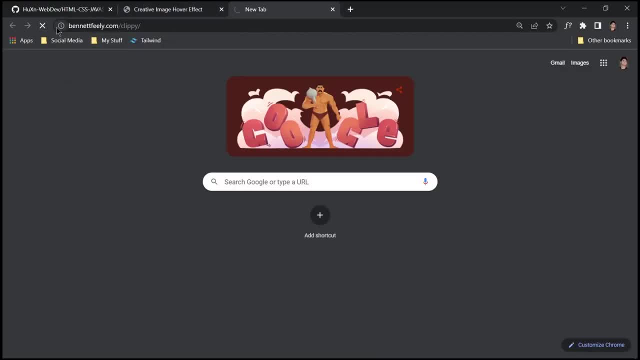 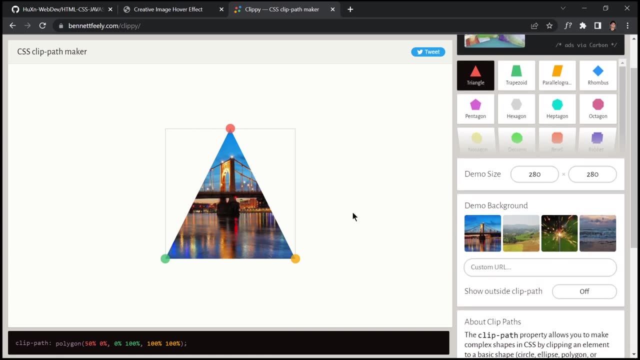 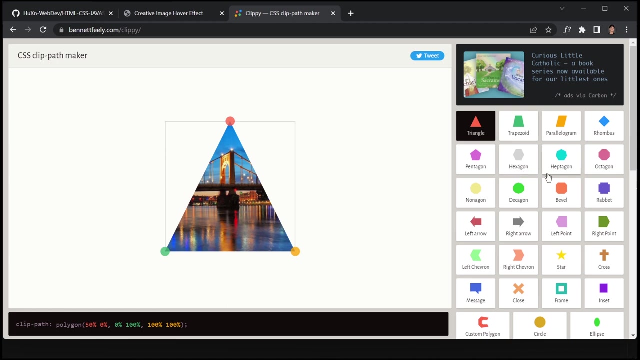 so if i copy the link of it and now here, if i click on that, i don't know- sorry, i can't pronounce the name of it, but this is the website. you can also find this website in the description area and here we can see it have a lot of uh clipping properties, like if you want to clip your image like um hexagon. 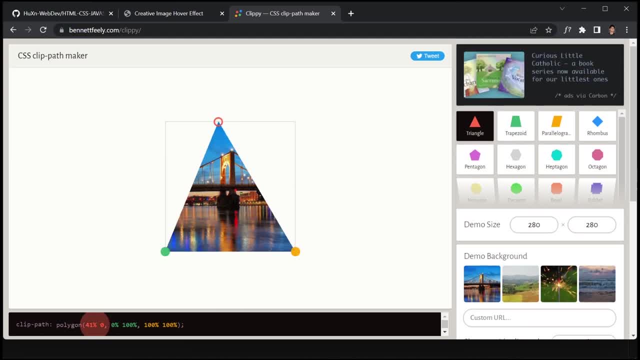 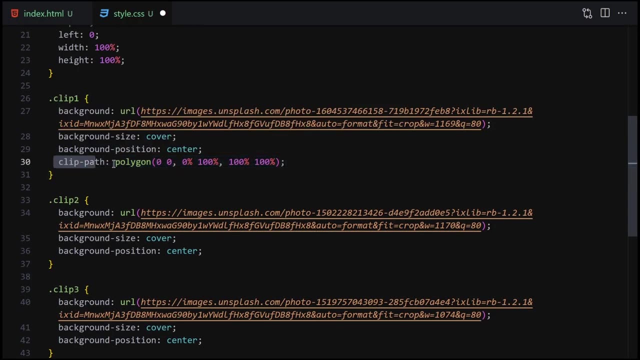 heptagon, octagon. you can do a lot of stuff with there, like you can just do it like so. let's suppose, if i want to make it like so, and now let me copy this clip path from there and then go to which yes or recorder, and i want to paste this link right here, like we have a clip path. 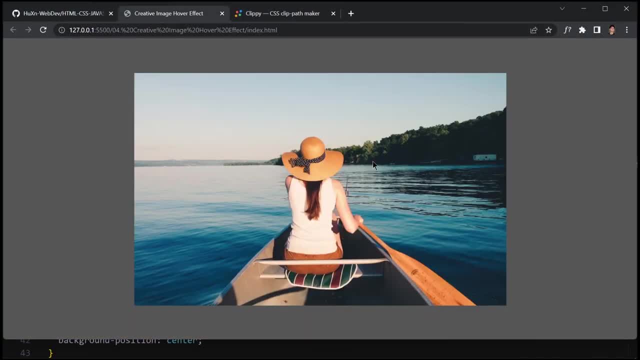 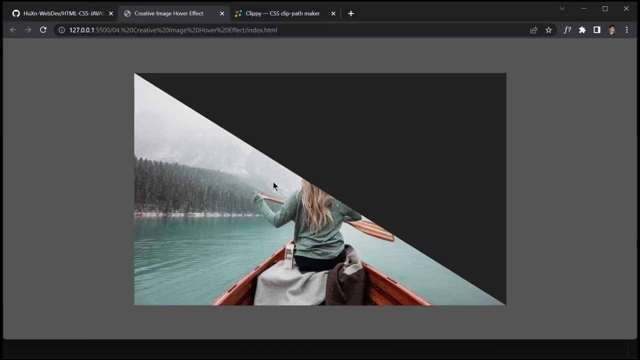 and then we have a polygon and one three zero file and here you can all see the uh. let me just comment out these images. so here you can see this image right here. so this image is now clipped like this. here you can see that. so if you want to clip it like i don't know, like a 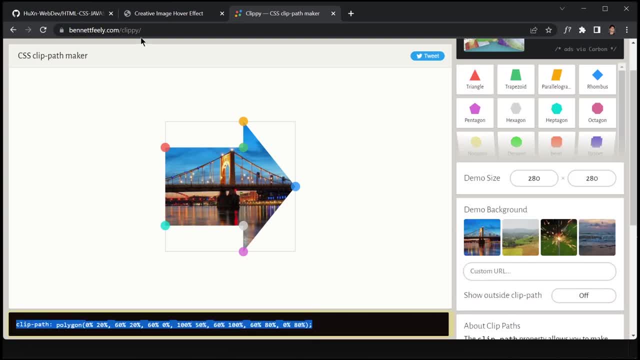 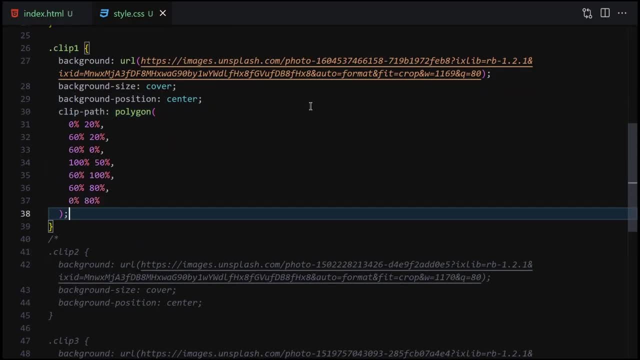 right arrow. you just have to copy this property right here in its value and then go to your side and then go to your terminal, uh, i mean like go to your resource recorder and just space there, and once we save our file- so here you can see- it will now, uh, clip it like the right arrow. 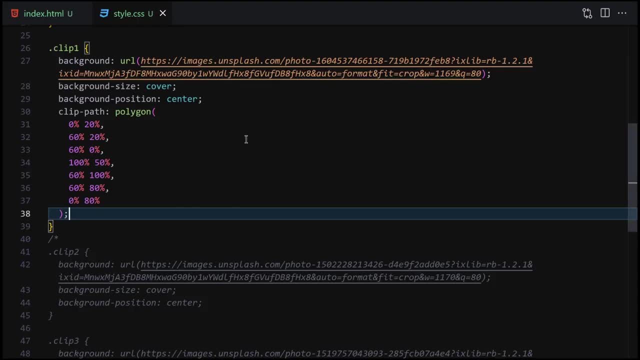 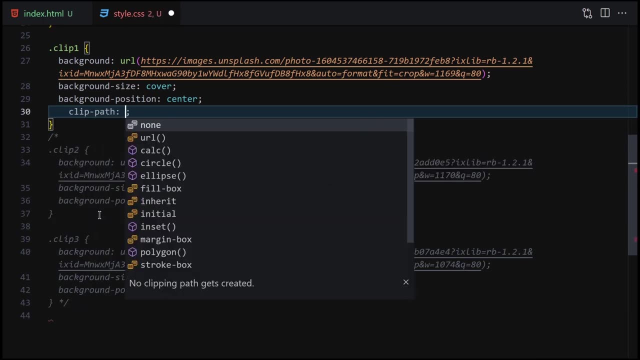 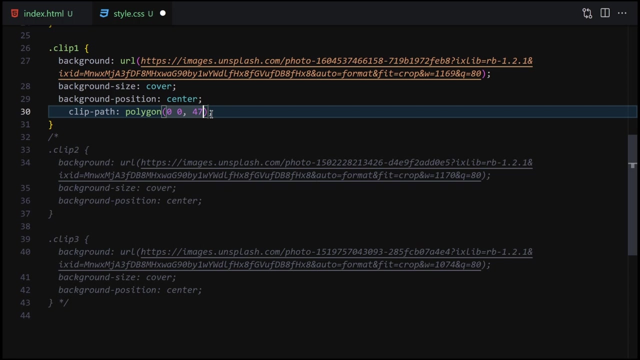 right here. okay, so you can play around with that. so i have specifically created a few properties for that, so i'll just remove all of that. then i'll just write like clip path and it will be set to polygon. so i'll just write like zero, zero for the first side and then 46 percent for the second side. 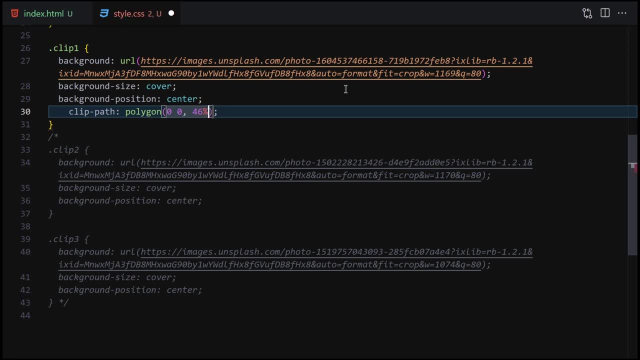 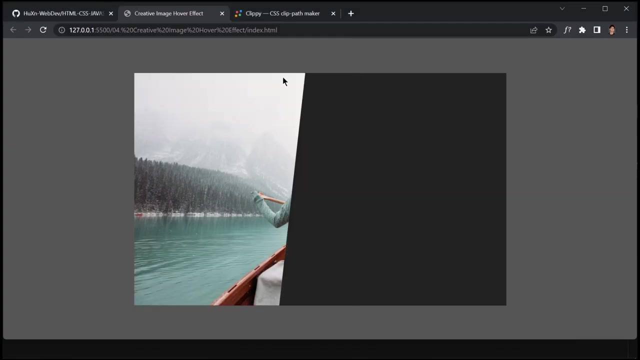 uh, just percent, not a dollar sign. and then i'm gonna hit, and then zero for the second side, and then 39 for the second, for the third side, 39 and 100, and then we have a zero and 100 for the right side. so once we save our file, so this is our first image. so now, if i uncomment these two, 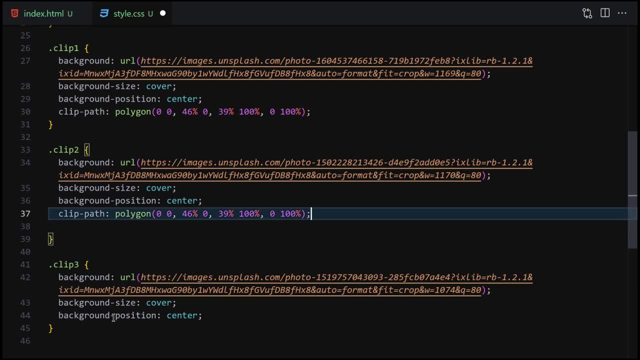 and then i'm going to copy this one from there and call paste right here and now let's change the properties of it to like: uh, i don't know, i'm going to change this one to 90 percent. i've already set there so you can play around with that, like, if you want to. and then 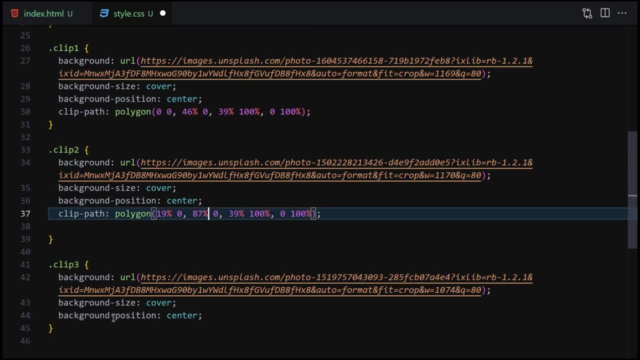 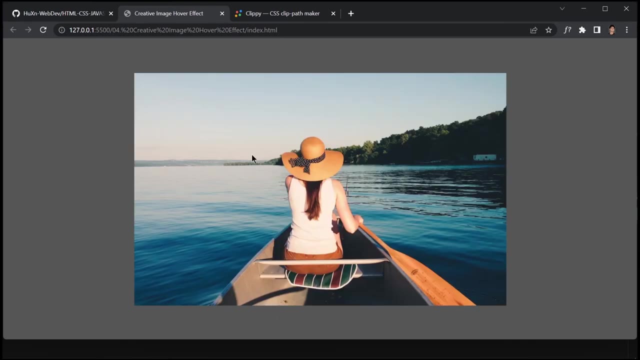 it will be now set to 87 and this will be zero, and then the third side will be 64, and 100 will be fine, and then 33 percent and 100 and once we save our file, so it really gives us the third image because we're going to set up this third image someone also pasted right here and now. 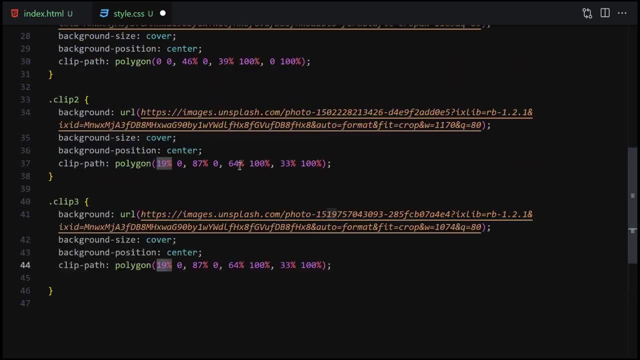 let's change this to like i don't know. i'll just change it to 37 percent, all right, so 82 percent and zero, and then we have like 100 percent color and 100 and zero, and then finally we have 100 and 100, and then we have 63, 63 and 100 and once we save our file. so this is currently now it's. 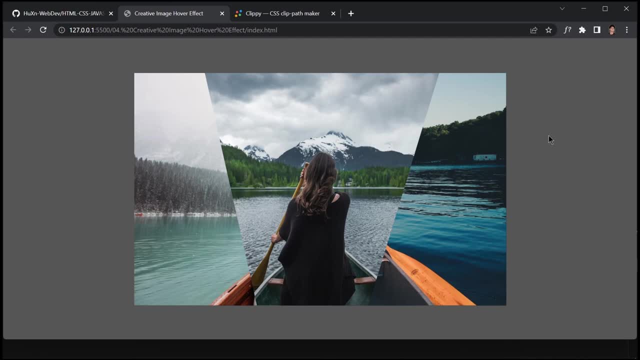 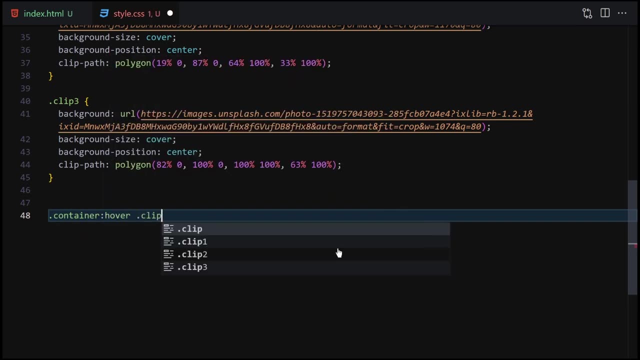 looking like. so now we have to provide a hover effect so it can do its thing. so i'll just write a container. uh, i'll just write a container and then, once we hover over that container and you want the clip path property and then we want to clip path of polygon. 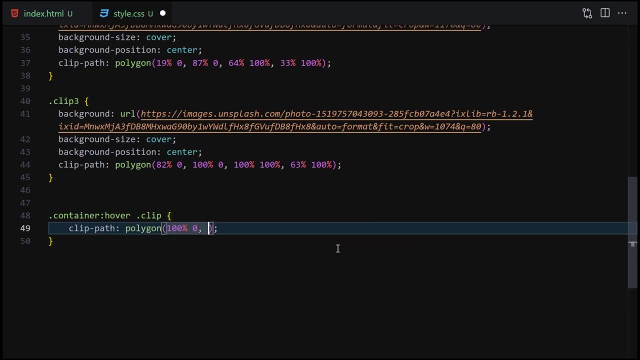 so the first property will be a hundred percent and zero, and all of them will be 100 and zero. so i'll just copy that from there. this is the first one, this is the second one, then we have a third one, and it will be: now equals two hundred percent, okay. and then we have a fourth one, which will be: 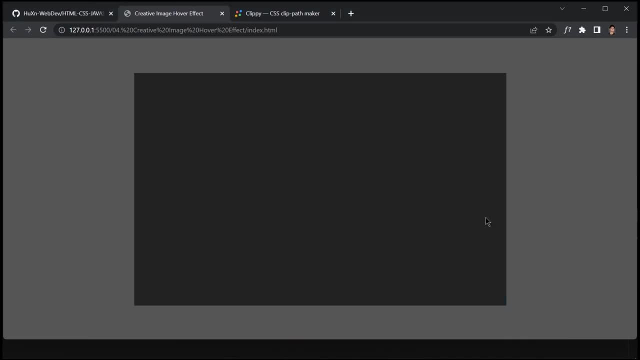 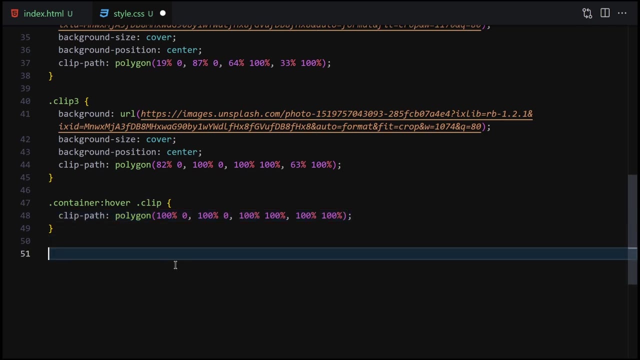 also hundred percent. okay, so once we save the file so we cannot hold water to it right now. all right, so it's now taking all of the space. so now let's select that other container and once we hover over that container- uh, not a hover, but once we hover over the clip of that container- and then we have to. 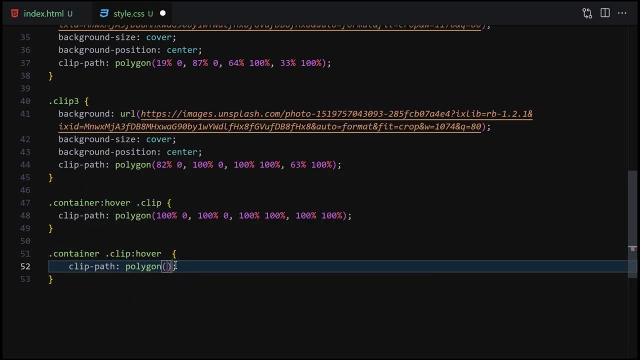 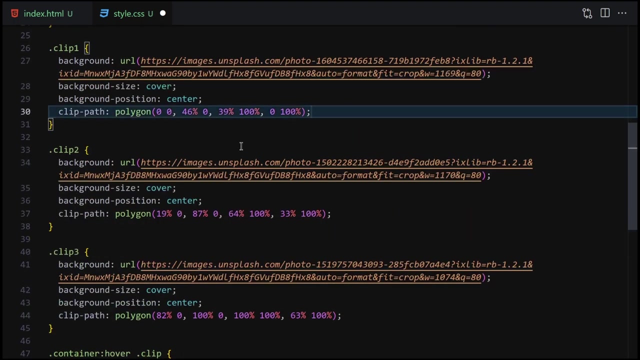 just write a clip path of polygon and then zero, zero comma, 100 comma, not comma, but zero comma, 100. so 100 percent comma, zero percent and hundred percent. okay, so now we have to add that right here, or transition. so i'll just write like our transition to this clip property. so just write: 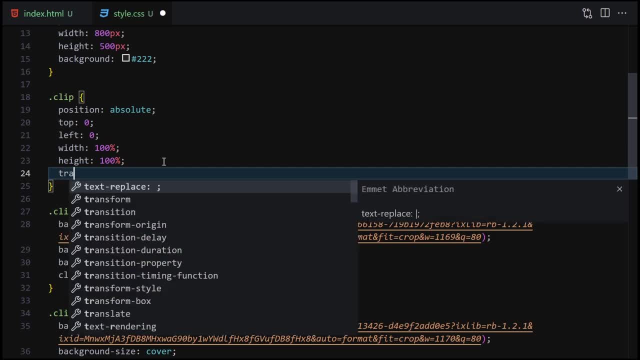 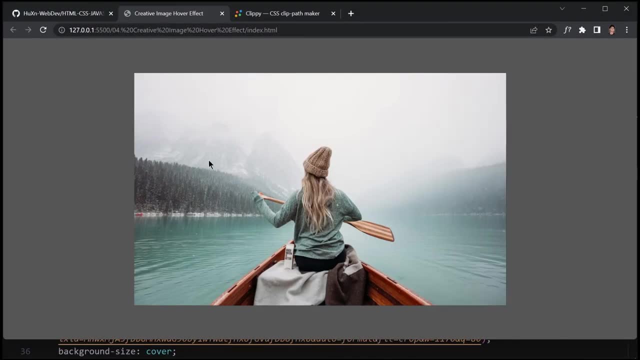 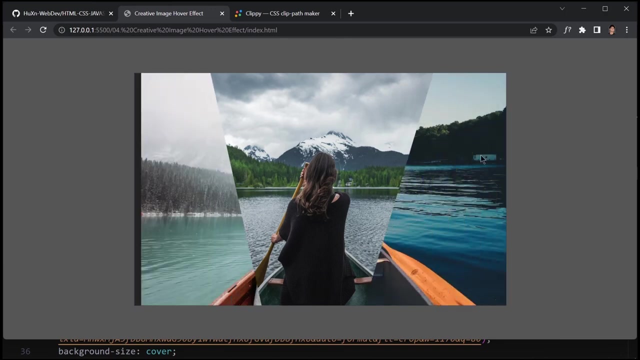 transition, not duration, but transition of 0.5 second. and once we save our file. and now, once we hover over to this goal, so it will take the entire space. once we hover over at the middle of the goal, so it will also take the entire space. and once we hover over to this goal, so it will. 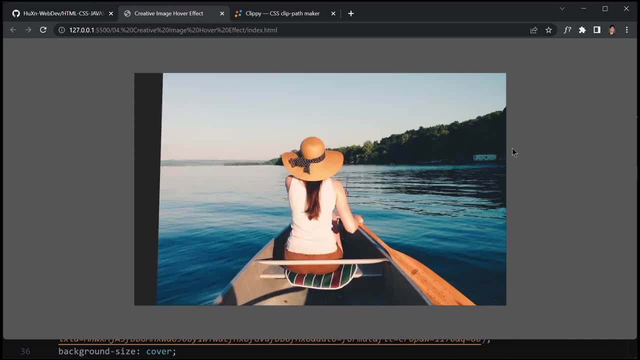 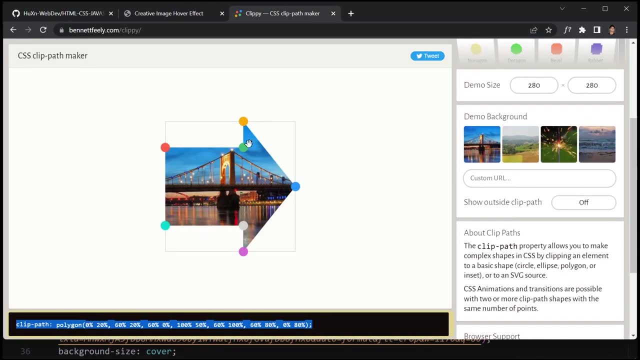 take the whole, the entire space to be precise. i can't even speak now, anyhow. so now you get this clip property. you don't have to swear about this property. you just have to mess around with it like i don't know, just grab these corners and then just like, mess around with it, so you get what's going. 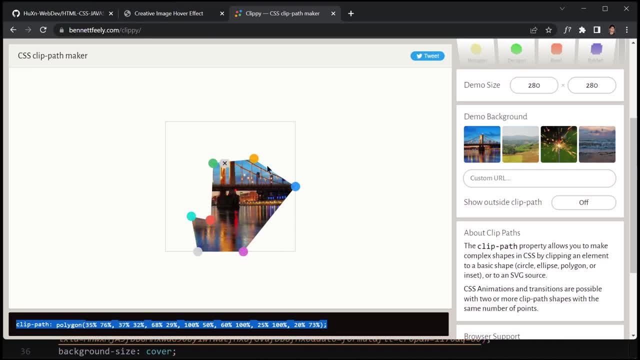 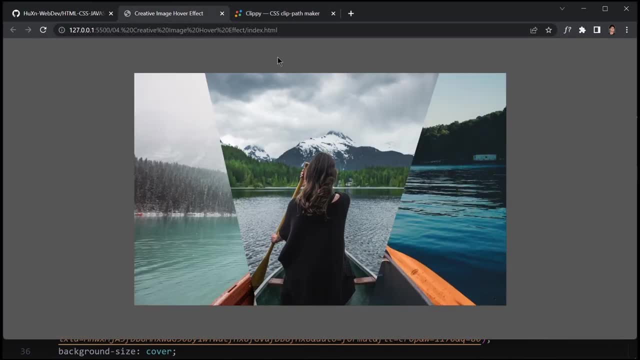 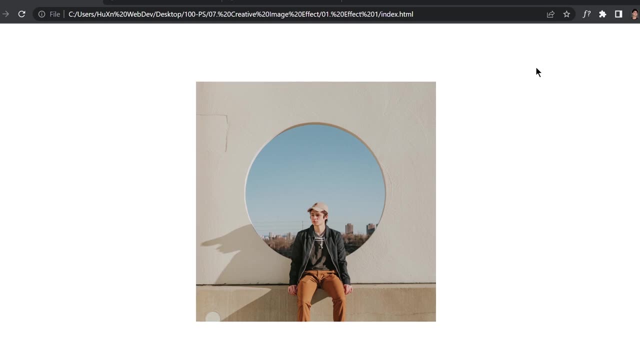 on okay, so i would recommend to just take a little bit of time with that. it's kind of like a twitter, i don't know. all right, all right, so that was it about today's project. hey guys, and welcome to the seventh project of this course. so in this for you, we are going to 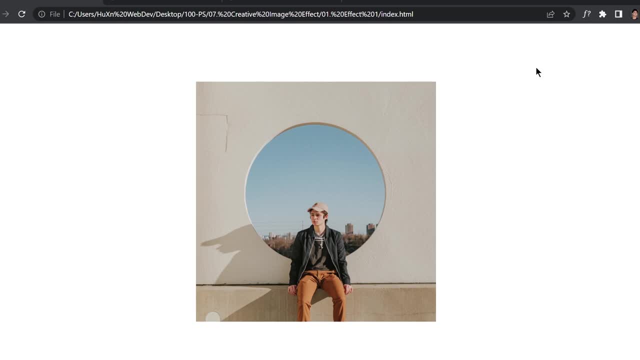 be creating a creative image effects by just using html and css. so the first one will be this one. so once we have our mouse over to it, so we would get this kind of animation right here, and if we move it, so we'll get our image right here. so now the second one which we are going to be creating is: 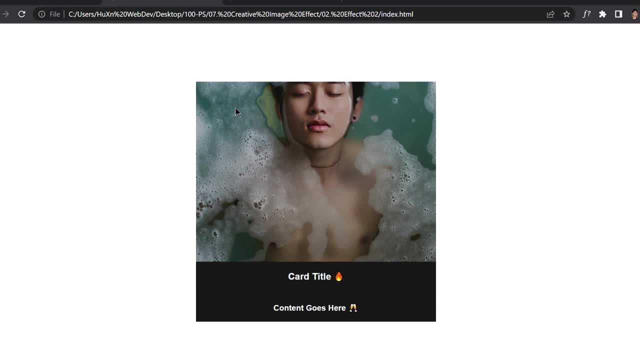 once we hover our mouse over to it, so it will now gives us this uh container right here at the bottom, and we are going to be creating a creative image effects by just using html and css. so we now, if we move it, so it will now gives us our image. so now the third one which we are going to be. 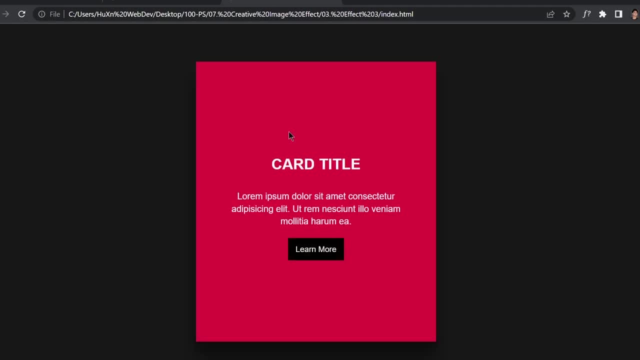 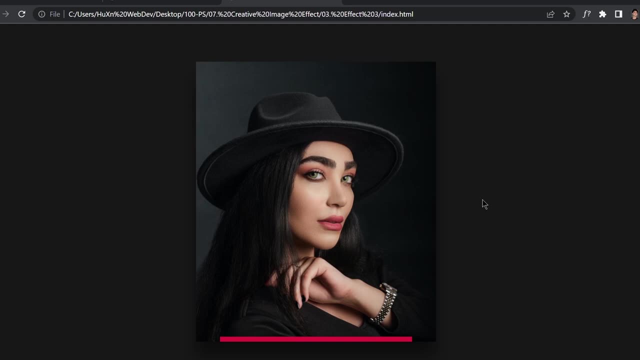 creating is once we hold our mouse over to it, so this container will take its entire space and we will have this content right here. so if you take one mouse off, so it will now just collapse right here. so we are going to be creating these three animation in this video. so now, without wasting any, 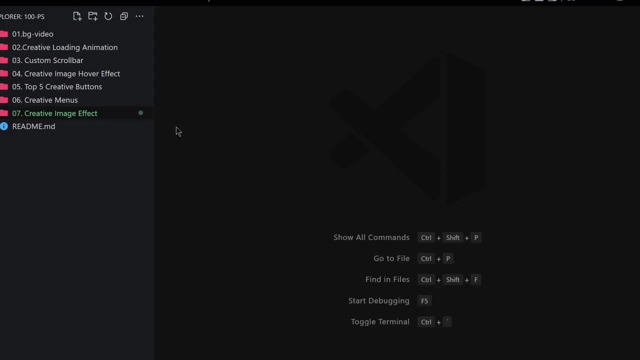 time let's jump right into our coder and write out code. in the previous video we've created this: creative menus. in this video we are going to be creating this uh, image effects by just using html and css. no javascript, no preprocessors like saas, etc. but just html and css. so in the description of 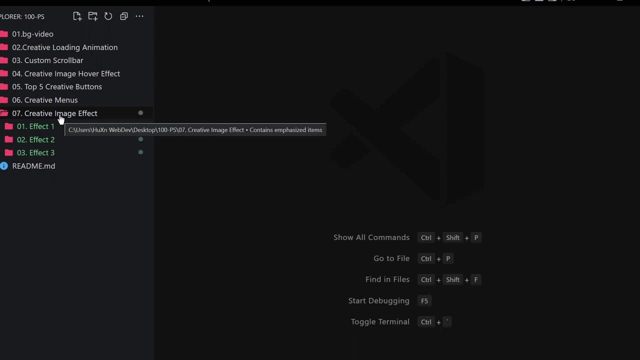 this video, you will find a link to my github repository, so i want you to go to the repository and download this folder. inside this folder, you will find three nested folders and no code. what so? i have like this indexhtml file in stylecss file, but no code whatsoever in all of these files. 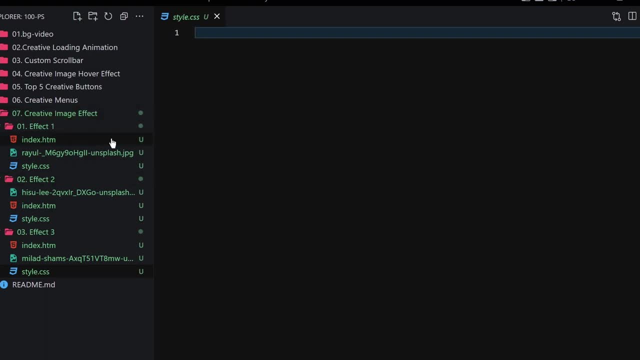 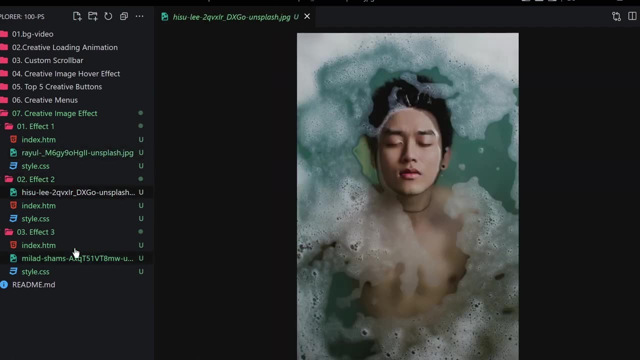 okay. so no code, nothing inside this file. you can create it by your own, but the thing i want you to grab is this code inside this code and you can use it in your physical files. so i want you to go three images like: the first image will be this one, the second will be this one and the third one will 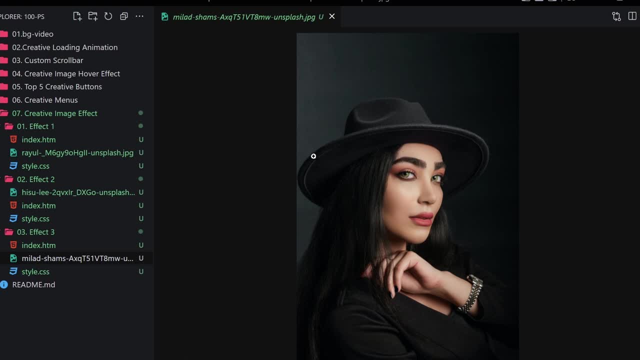 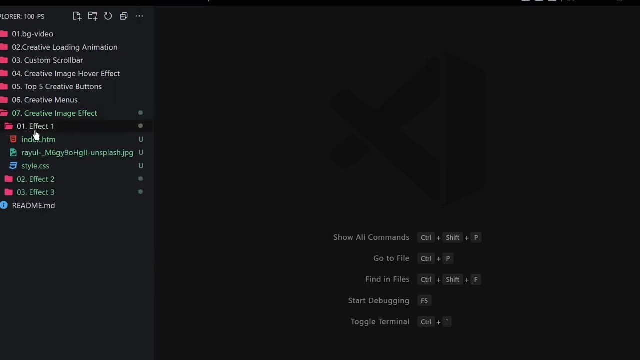 be this one and again, you are totally free to use your own images if you want to follow along with this video. so you can just uh download these images from my github repository. okay, so starting from the first one, which is their effect one, i'm going to just open my indexhtml file and start. 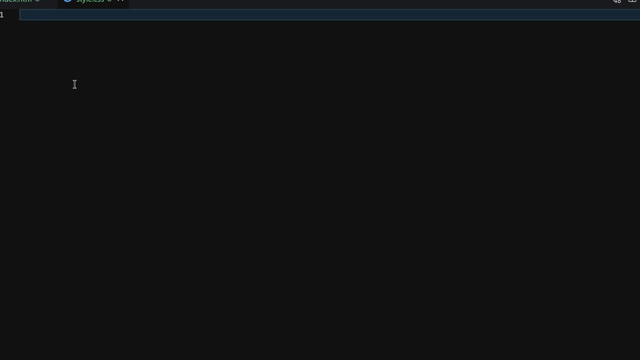 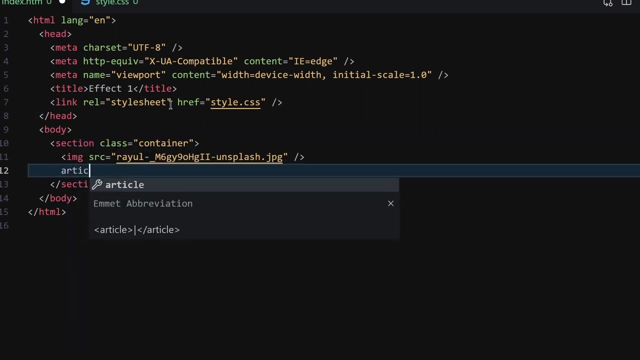 our css file. okay, so now let me zoom in a bit so that you guys can see everything a bit better, and then i'll just write a doc and here i'll give a name of like effect one, and then i'll also link it with my css file right here. okay, underneath this image we can write our article and this: 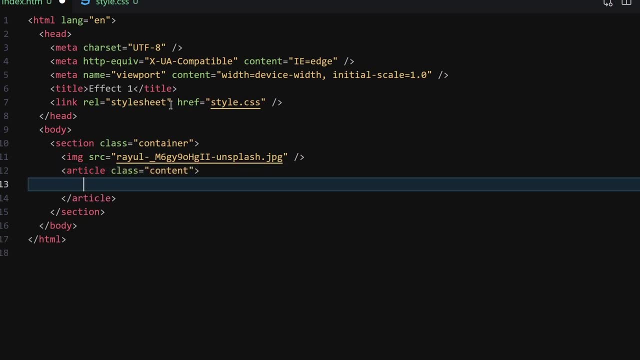 article will have a class of content. okay, inside this article we will have like h1, which will say like: welcome to the uh, the real world. and then we will have our h4 and which will say like: write your uh content here, uh content here. or you can choose emojis. if you want to grab emoji, you just have to hold. 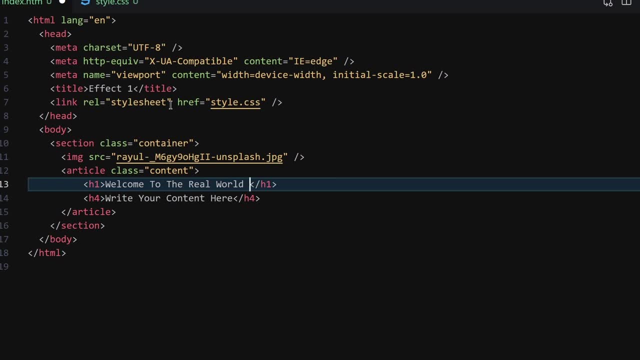 the windows button, or i don't know how to work with the mac, but in windows you can just hold the windows button and then just hit period or dot. so then here you can choose, like whichever emoji you like. in my case i want to just search for like: uh, i don't know, s would be fine, and then 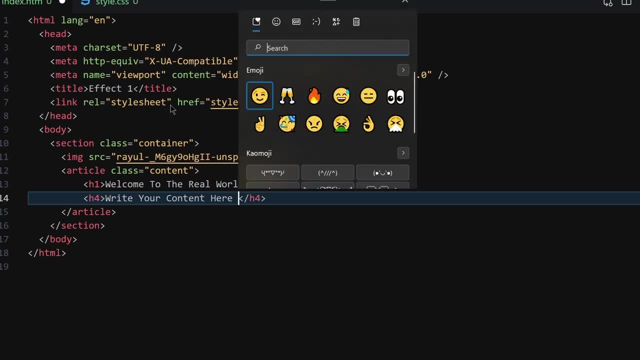 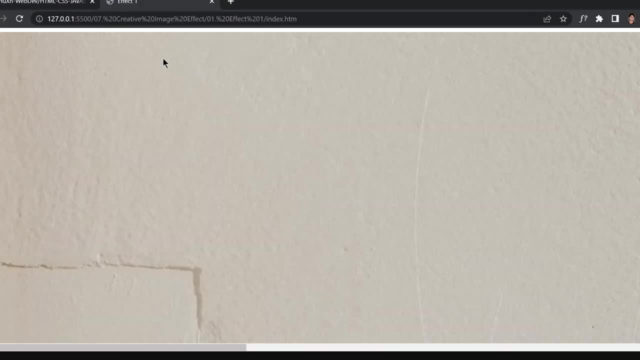 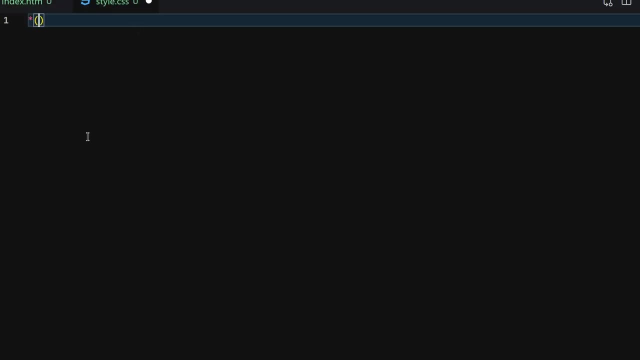 i'm going to click on there, i'm going to choose that one, and then these glasses will be fine. so once i save my file file, then i have to launch it by using a live server. so here is my image right here, really massive- and here's the content. all right, so then i want to go to my style sheet, and first of all, 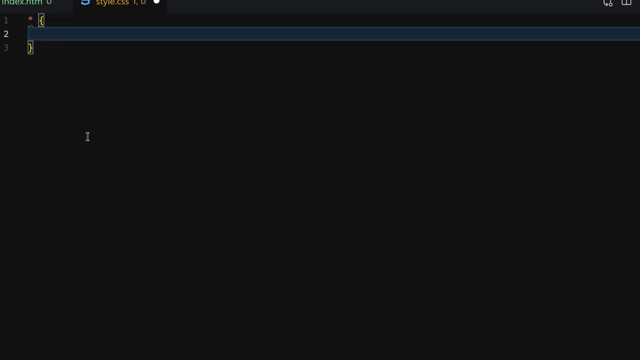 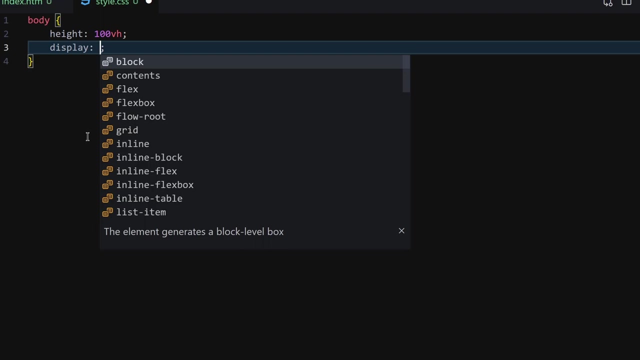 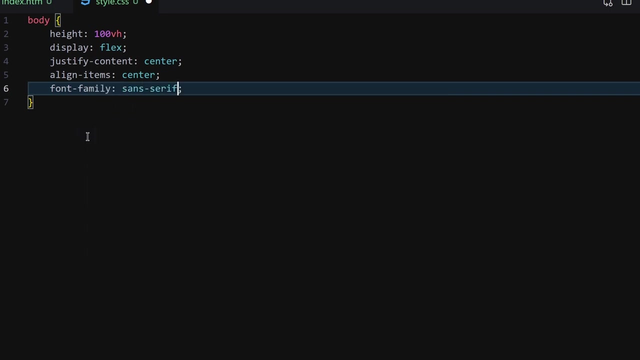 we are going to be writing our research, so, uh, you know i'll just leave the research for now. then i'll just write: body and height will be 100 vh. display will be flex, justified content will be center, aligned items will be center and farm family will be sensor. you can choose whichever. 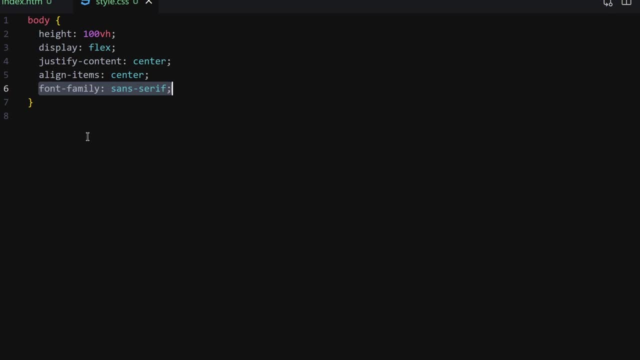 farm family, you like, but in my case i just choose like sensor because it's simple and it will just remove those serves. okay, so, and i also want this to be like 100 vh and i want everything to be center, perfectly center. okay, so, everything is now perfectly center and this image is really massive. 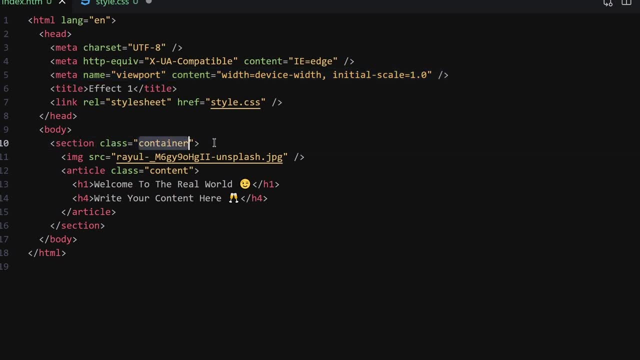 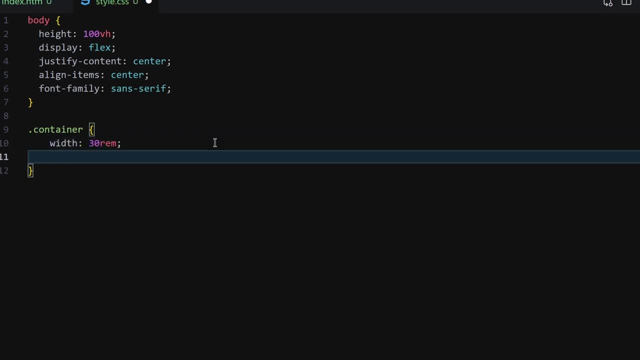 so first of all let's style this container and then we can take care of the other stuff. so i'll just write a width of 30 gram and then i'll also duplicate it and change the height with 30 ram, position will be relative and overflow will be hidden, so once i send my file. so here you can see, we've got this box, but 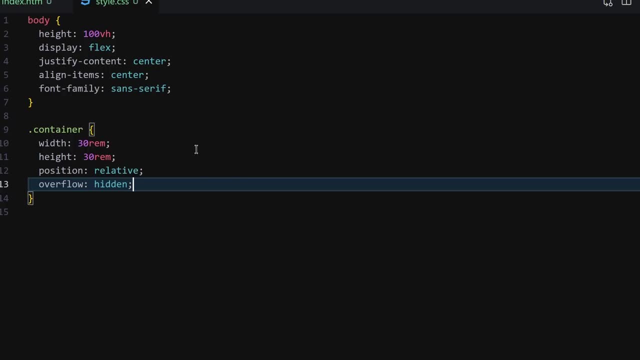 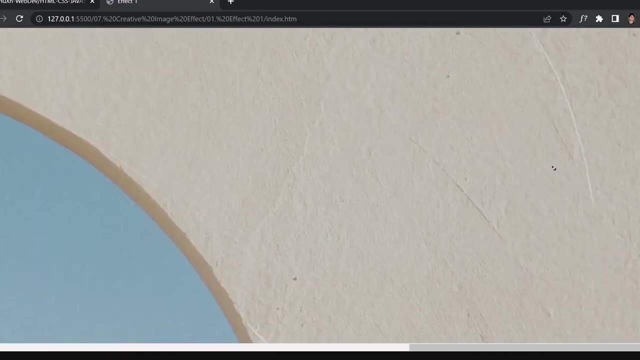 it's containing all of our image and all of our content. the overflow is hidden, so that's why we are getting nothing. so here you can see. if i delete that overflow, so here you can see that it will give us that massive image right here. okay, so overflow will be hidden for this case. 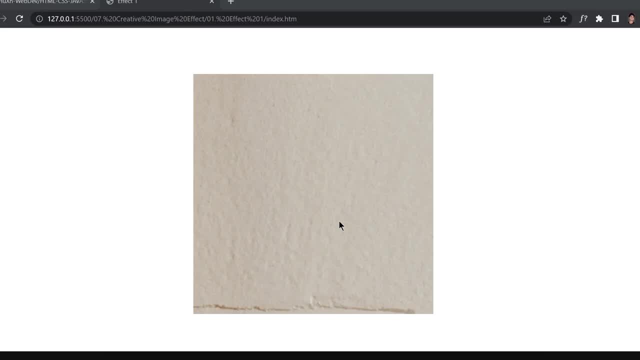 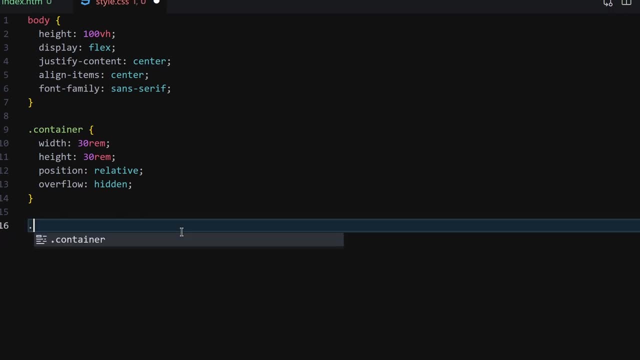 so, once i save it, we've got our perfect box right now. all right, so the next thing which i'm gonna do is i'm gonna select this image for now. so inside the container, um, inside that container, we have the image. so now let's select our image, and we want to give it a width of 100 because we want. 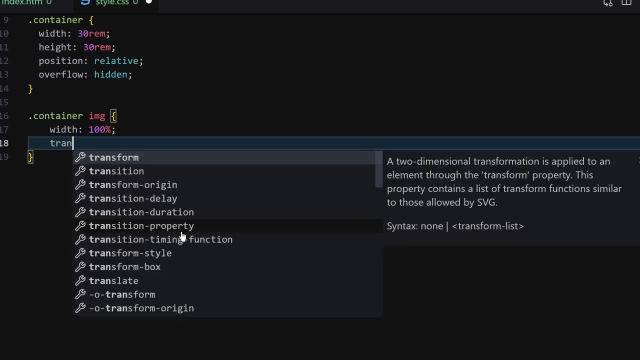 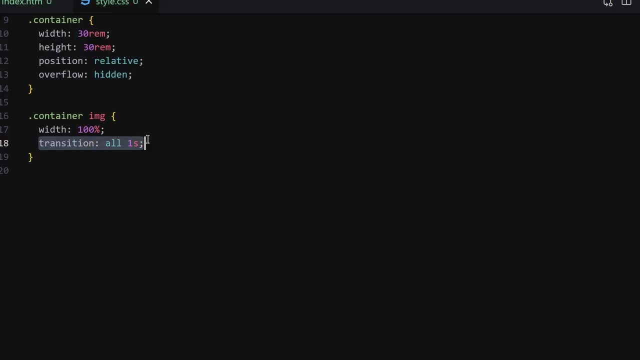 to take all of the entire space of the width and then transition will be one uh all one second. so once we sell a file, so here's our image. and we did provide a transition to it because whenever we are hovering over through this image we will have that other slide effects. so we want the transition to 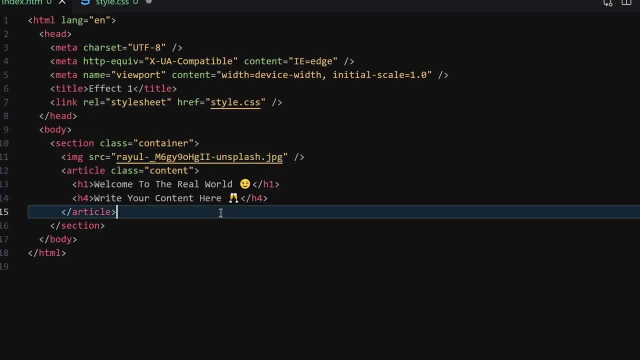 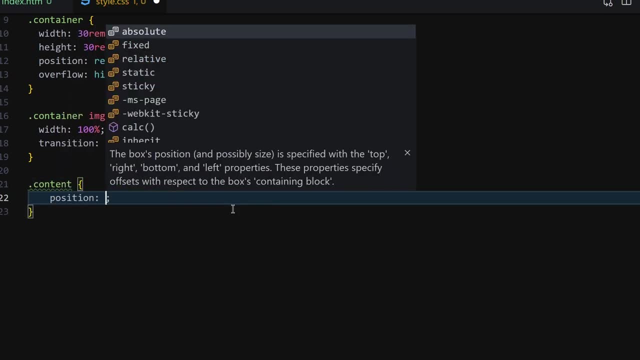 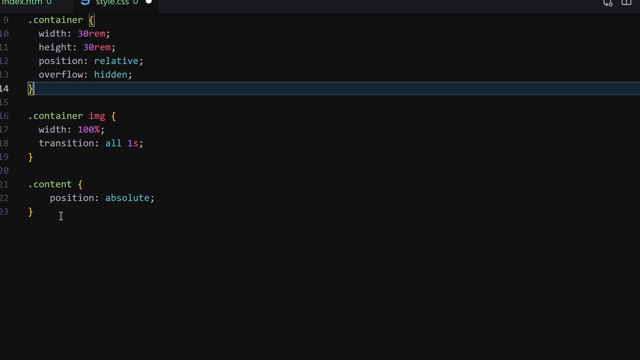 happen smoothly, okay. so the next thing which you have to style is this content area, so i'm going to just select like content and then inside this content, position will be now absolute. this one will be position relative and this content will be absolute to this container. okay, which means like. 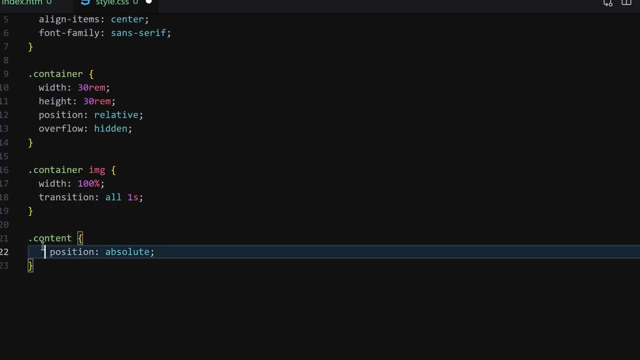 this content. whatever we do inside this content, this content will be nested inside this container. okay, so this is position relative and this is position absolute. and now inside, the top will be zero, left will be also zero and height will be 100 and the width will be also 100. okay, so this is our. 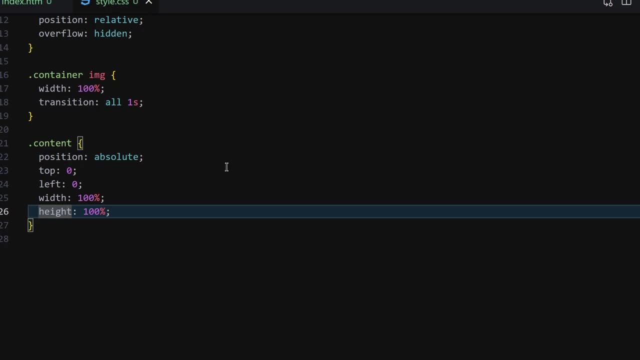 content right here and we don't have any hover effects, so that's why we are seeing that right here. and the next thing which i'm going to do, i'll just center the text inside this box right now, so i'll just write like: display of flags: justify corner center, align items of center. okay, and color will be totally white. 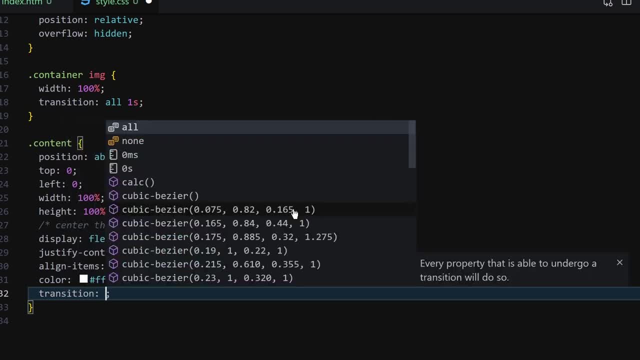 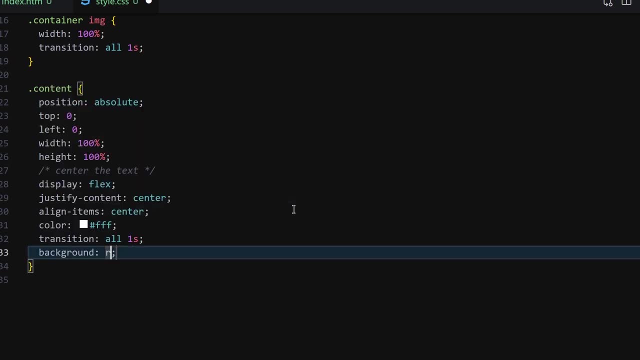 and then what i want to do is i'll also provide a transition to this one as well, because we will also provide a hover effect to this one, and uh, background will be rgb, and i'm going to change this one to 23 comma. and you know what? i'm going to copy this one and paste it three times, right? 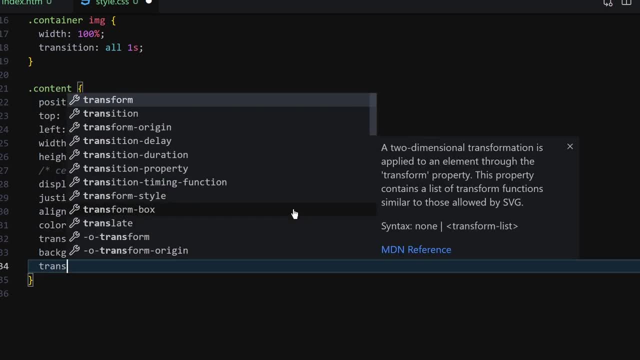 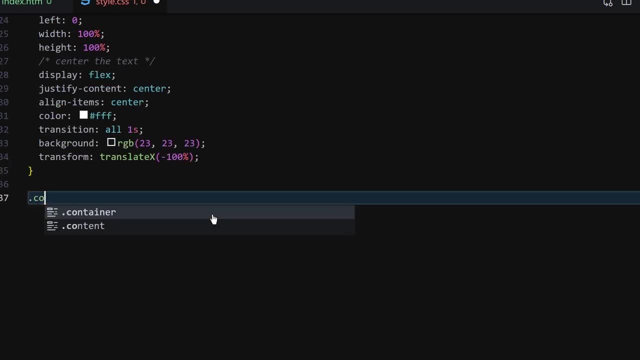 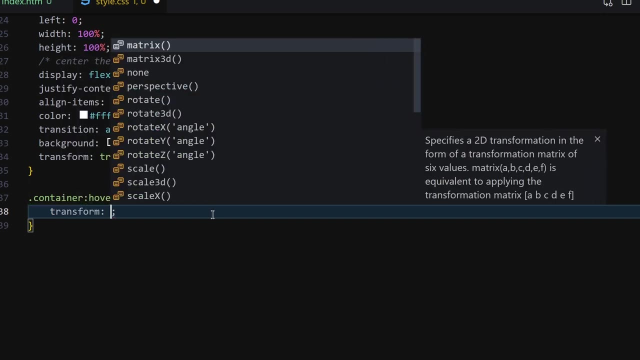 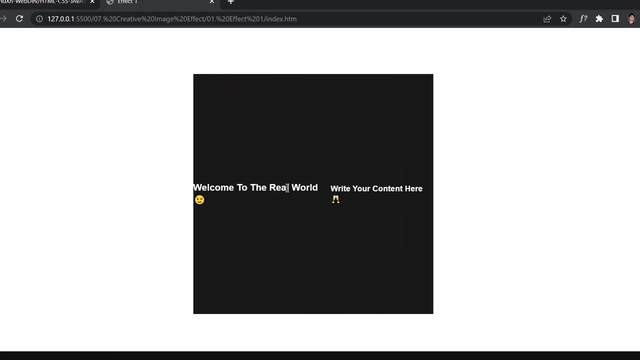 here. okay, so this will be my primary color, and then transform will be just translate x minus 100. okay, so now let's add our hover effects, so like content hover, and then i mean like container, however and content, and then transform will be translate x 0. so once we save our file and once you hold our mouse over to it, so here you can see our content. 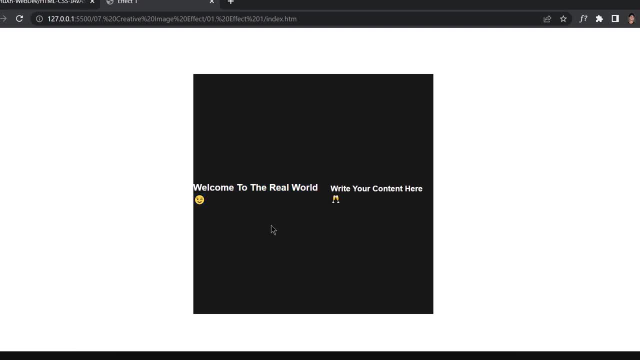 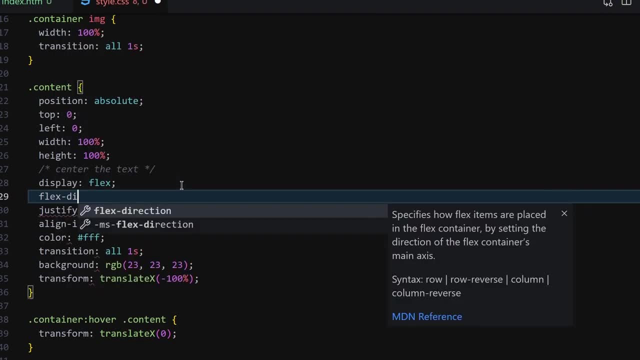 is showing up, but this is looking a bit messy. so now let's start that. okay, so let me just provide a justify- not justify, but flex um, direction the column and save my file and whenever we have our mouse ordered. so this is how it looks like, okay, and the last thing which i'm going to do is i'll also provide a hover effect. 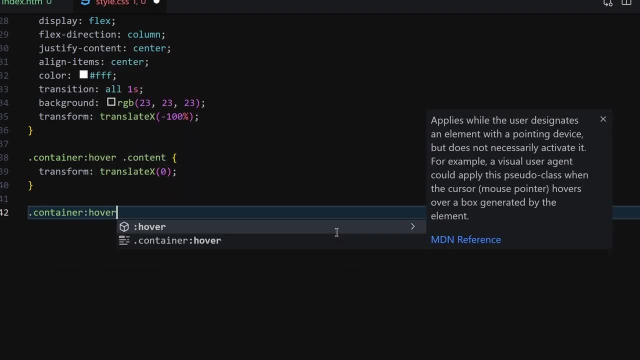 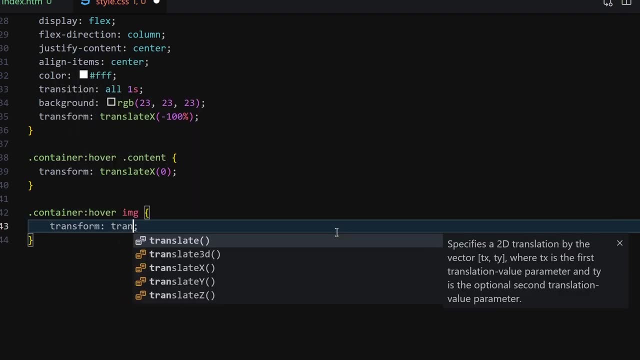 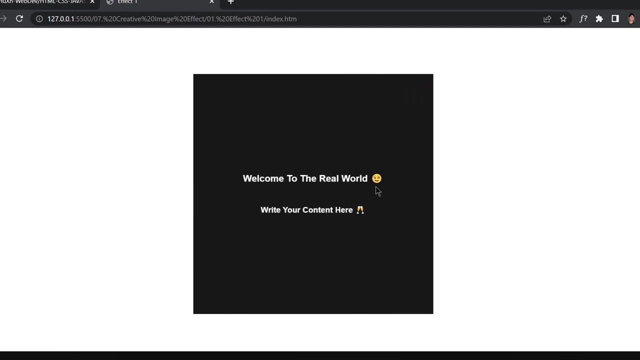 to this image. so i'll just write container hover image and then transform um transform to just translate x hundred percent- and save our file. so whenever we have our mouse over to it, this image will be gone and then other slide will take its place. okay, so if i just comment that out, so it 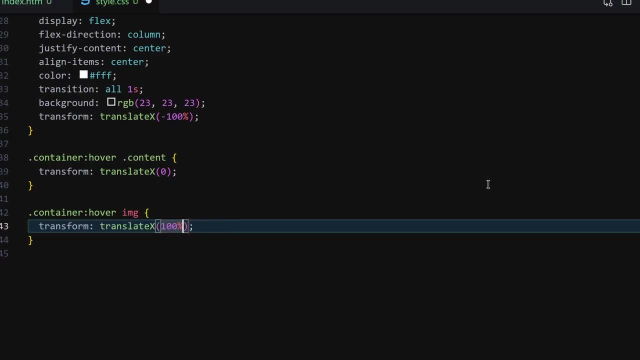 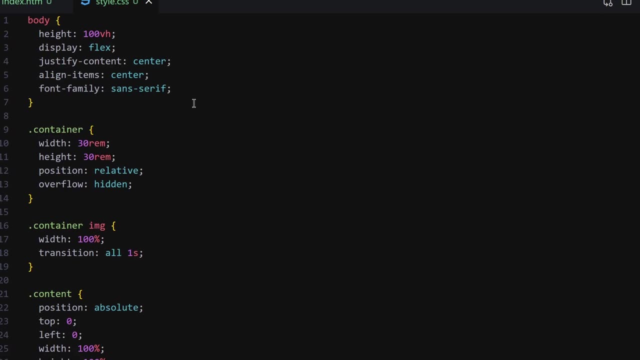 will just happen smoothly and this will not push up to the right if we uncomment it and save our file. so it will now go to the left and this one will also take its place. okay, so this was the first effect. we just styled the body, we just styled the container, we styled the image. it's 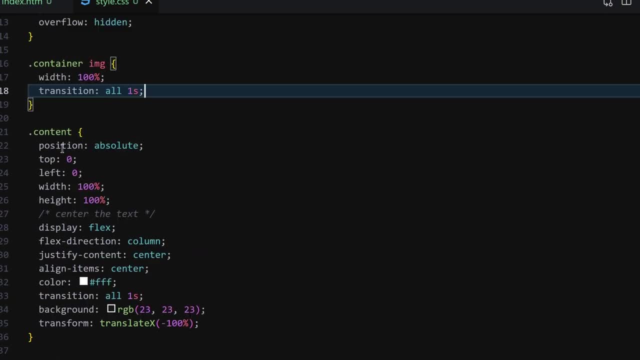 smaller and we just provide a bit of transition to it, and then we're going to do the same thing. we just set this position to absolute: top will be zero, left will be zero. we provide the width as same as a container, and if we just center all of our content. so this was the second slide and 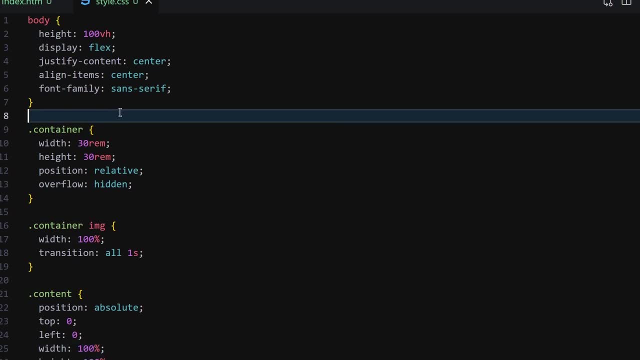 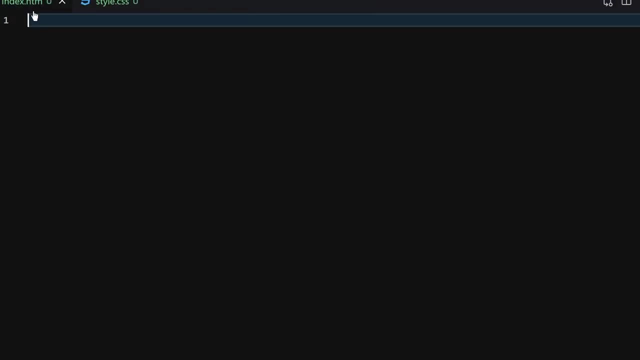 then we just provide a bit of hover effect to it. so that was quite simple and easy. so now let's jump right into the next effect, which is this second one. okay, so i'll open both of these file, and here i'll just try like doc, type html and effect 2, and then i'll also link it with my css. 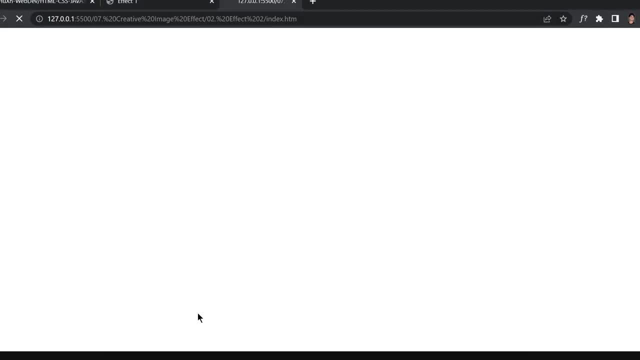 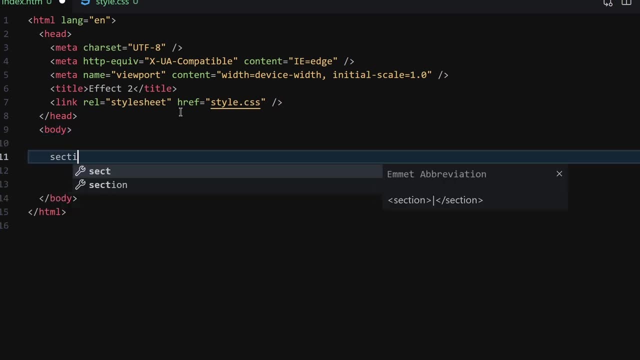 and i'll also open it with the live server. and now, here for the html side, i will just write like: um, it'll be the same as the other one, like section. we have a container inside this section. we have a image which will be this girl image or the boy, i can't remember. and then we have article. 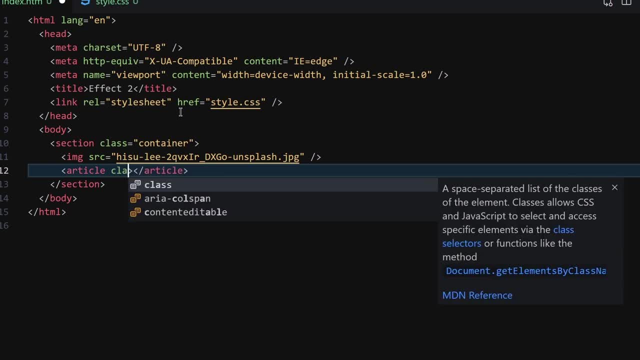 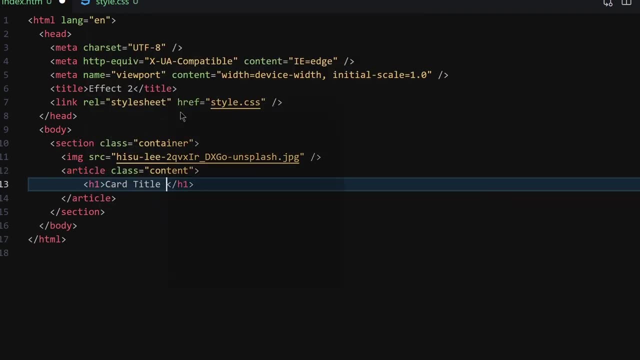 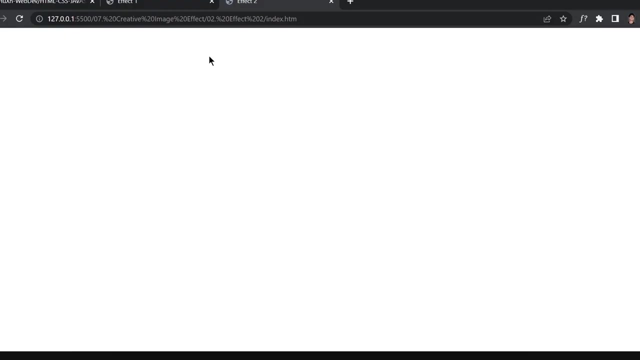 and inside we will give a class of content and inside this article we will just write h1 of card title and then- uh, i don't know your card title, maybe this emoji will be fine. and then you have h4 which will say: like content then goes here and then we'll just choose this glasses emoji cell. 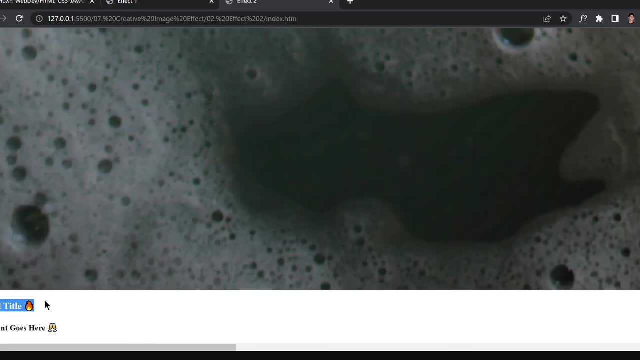 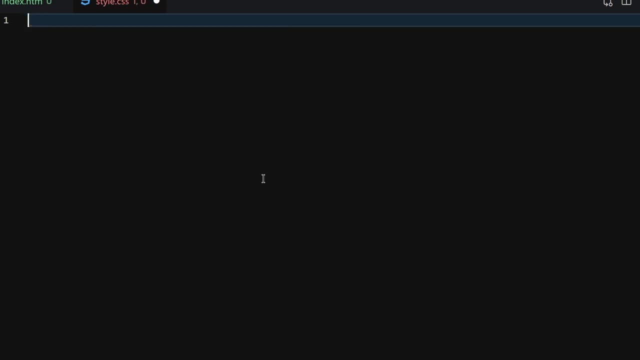 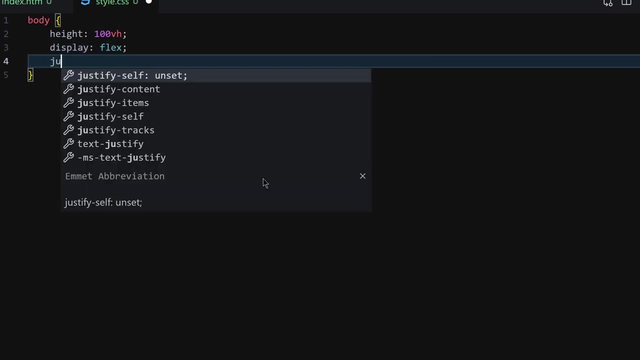 file and this is our image and this is our content right here. okay, so now let's jump right into the css and style it a bit. so first of all, i'll just do like a perfect centering, like body will be 100 vh. um, and then we have a display of flags, justify content center, a line item center, uh. 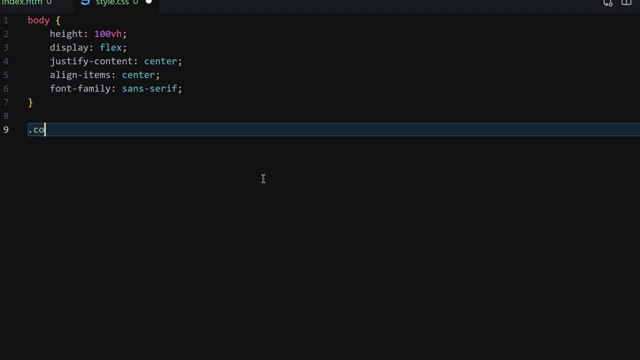 phone family sensor. if you can choose whichever phone you like, then i'll select my container, which will be 30 ram and height will be uh, also 30 ram, and position will be position will be relative and overflow will be hidden, as we saw just in a second ago. so it gives us this box right here. so 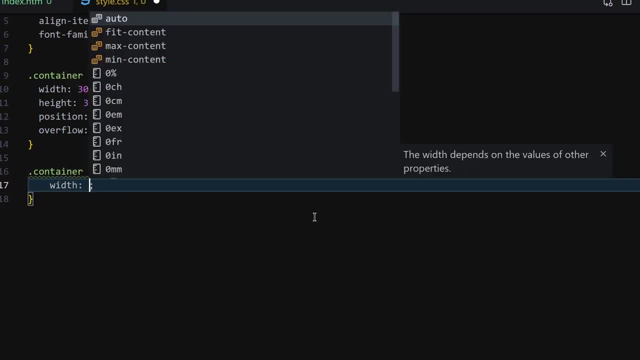 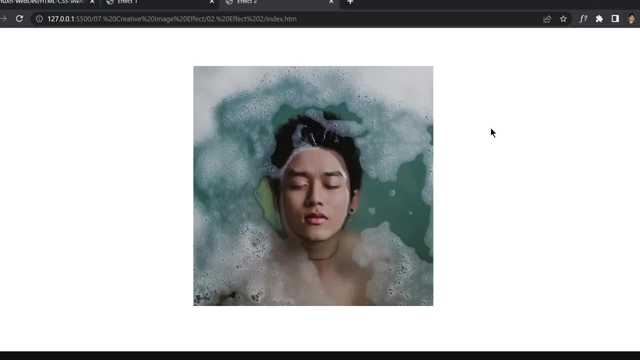 select our container one more time and image inside the container width will be 100 and transition will be all 0.5 second, and once you save it, nothing will shows up except this image will be perfectly centered inside this box. all right, so now let's jump right into the content. 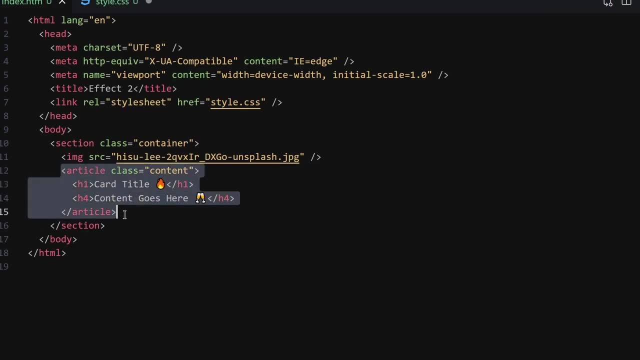 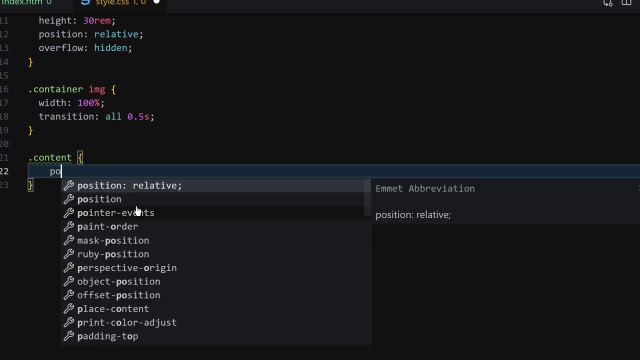 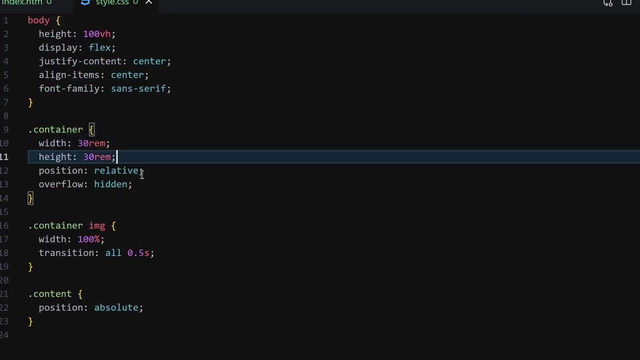 area, which is this content area. like we are going to be selecting this article and this content inside this article, so i'll just select this content inside this content. position will be selected and we have a list of content that we want to be centered inside this container. 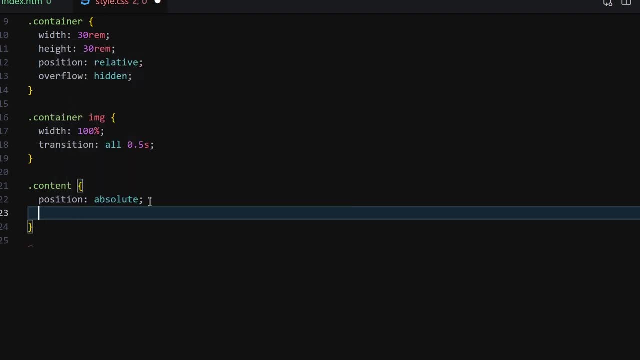 okay, so this is a position relative and we want them to be like position absolute. and then bottom will be, bottom will be zero and also, uh, left will be also zero, and then we have a height of 25 and then width will be 100 percent. okay, so once we sever it, nothing is going to happen. and then let 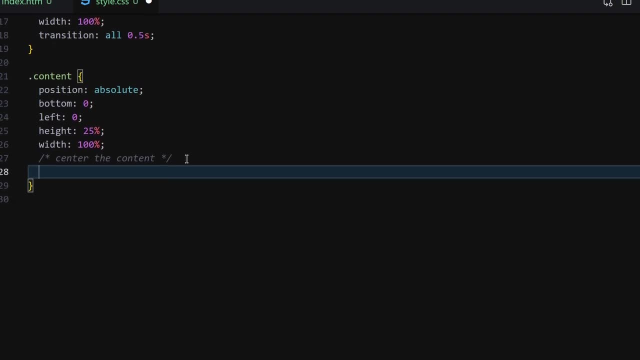 me: center the content, whatever you want to call it, and then just write a display of flags: justify corner center, align- um, okay, uh, flex, direction will be column. justify content center, align item center, and then color will be totally white and also we have to provide a transition to it. um, all 0.5 seconds, and then 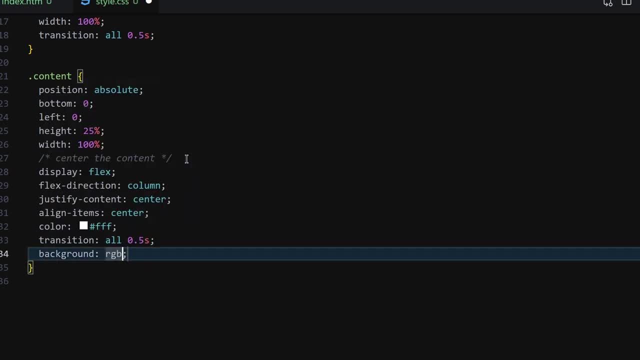 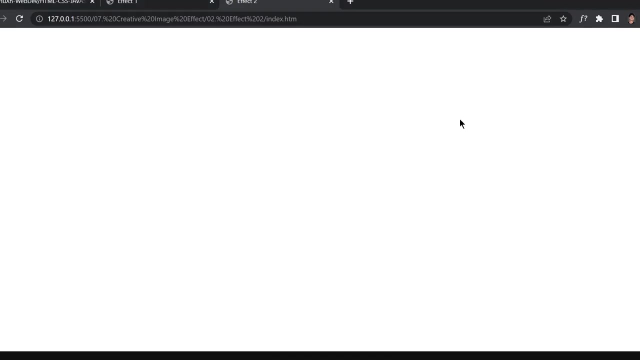 um, background will be just rgb, rgb, and then, uh, 23 comma, and let me just copy that and paste it one more time and one more time and remove that comma from the end and then transform, translate, y axis and 100, so save it and this is our content, right here. okay, can you see? okay, let me just 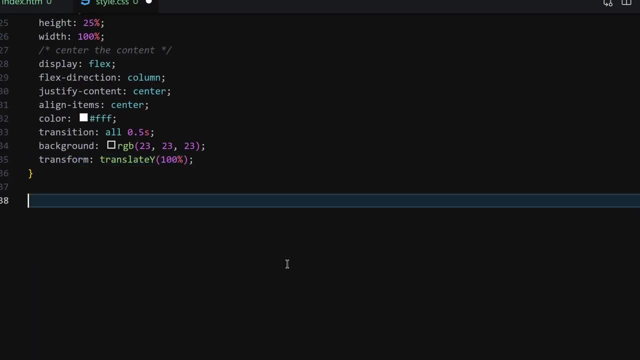 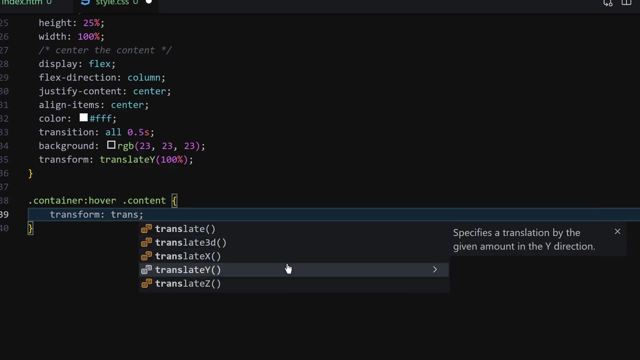 wait a bit. all right, so content has gone from there. so now let's provide our hover effect here. so container, and whenever we hover over to this container in content, not container but content. and here we'll just provide a transform of translate to the y-axis and zero percent. 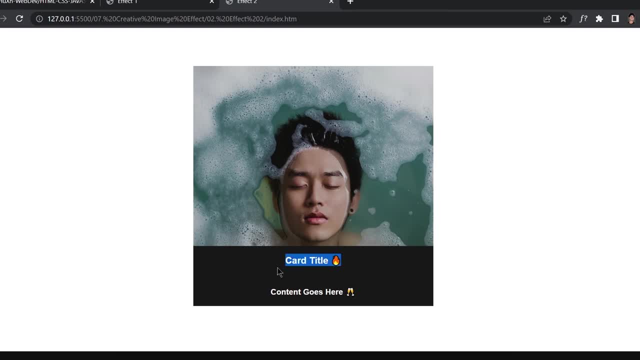 so once we hover over to it. so here now you can see we have this card title right here and you can just write your own content right here. okay so, but this image is not going up above, so you want this image to go a little bit above and also this, uh, this content container as well. so now let's. 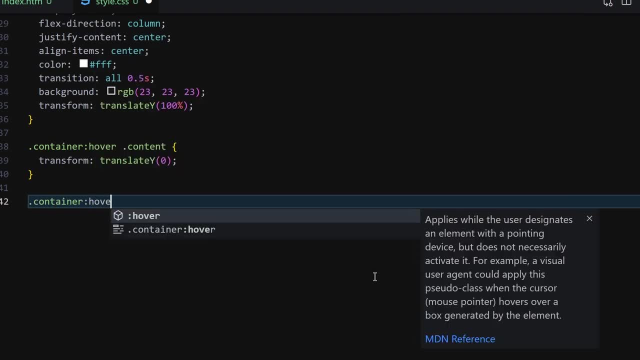 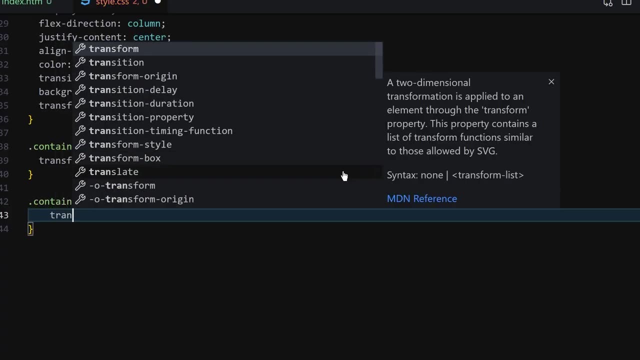 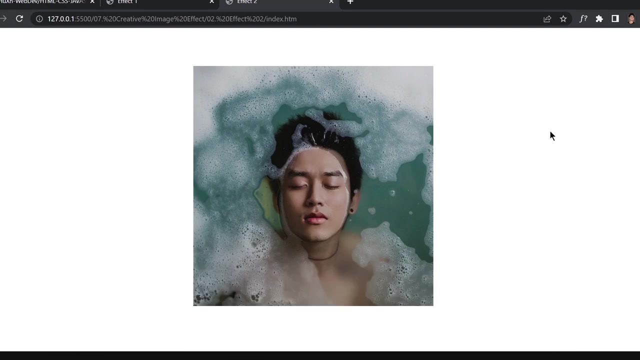 do that. so for that we are going to be using container and then hover image. okay, so whenever we hover over through this image, so this image will just push itself to a little bit above. so we will just write: transform, translate to y minus 30 percent and save our file. and now, once we hover, 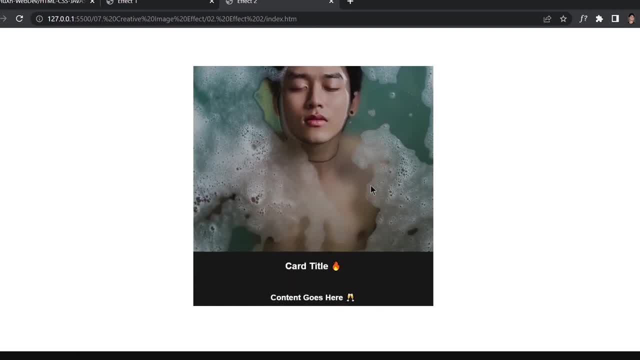 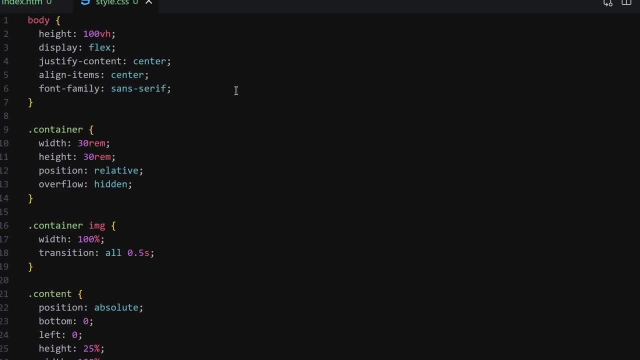 over to it. so here you can see this image is getting above and also this content area right here. okay, so this was the second effect, so now let's jump right into the third one. let me review all of this code as well. so we are just providing 100 vh height and we are just perfectly centering our 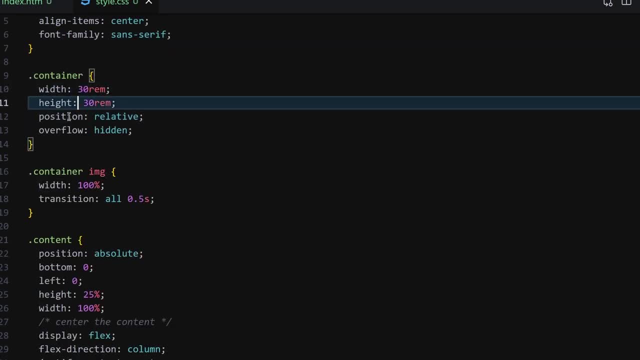 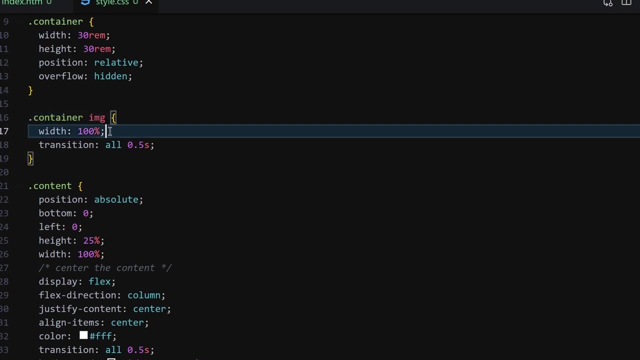 container. inside this container, we give them a 30 vh height and width and position will be relative and overflow will be hidden. and then we have a container. we select image, we give them like, the same width and height, like tag, the same width and height of this container, and we just provide a. 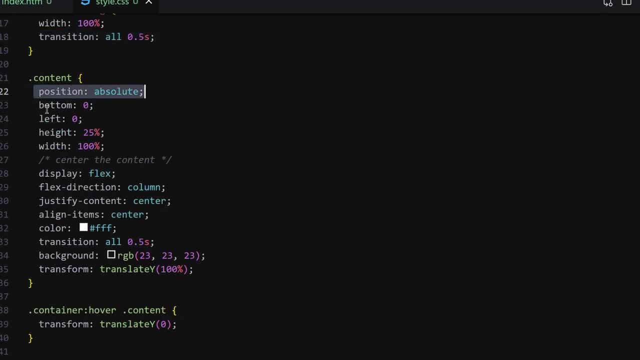 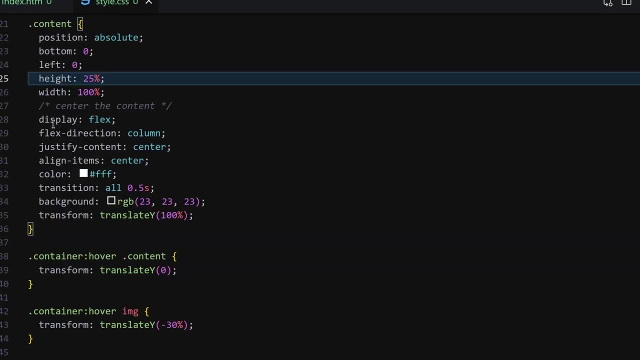 little bit of transition to it. then we have our content. the position will be absolute bottom left, everything will be in zero percent and we will just provide a little bit of transition to it. and then height will be 25 percent and width will be 100 percent. then we center what text inside? 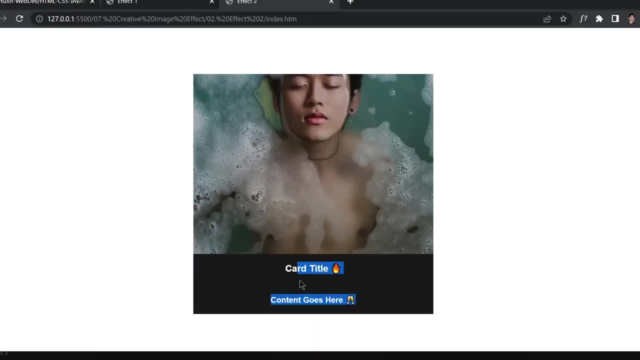 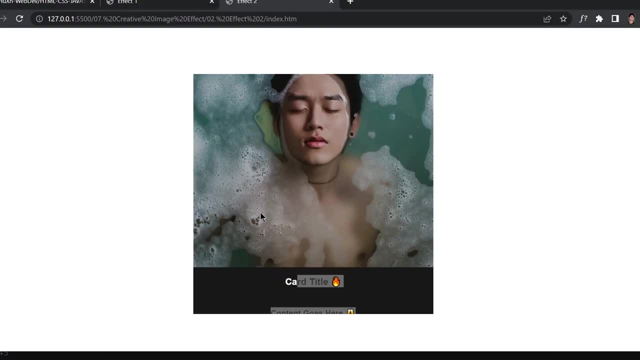 that container, inside this little container here, you can see that- and then we just give a color wire transition and then we just give a background of that kind of black color right here, and then we also provide to transform. translate y. so whenever we hover over to it, so it will just. 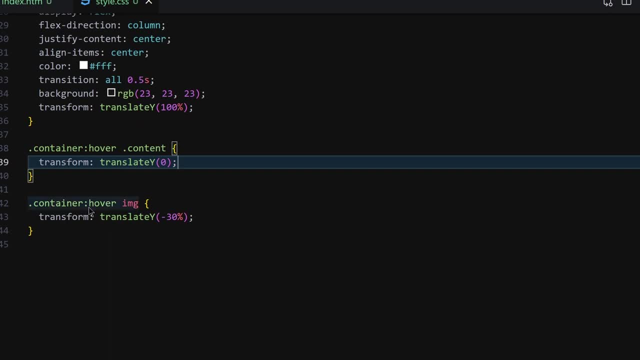 take its place to us from zero to 100, and then we provide that same transition to the image. so once we're done with that, we can just go ahead, and we're going to go ahead and we're going to go over to it. so it will just translate to the y-axis for like minus 30. okay, so this is how it looks like. 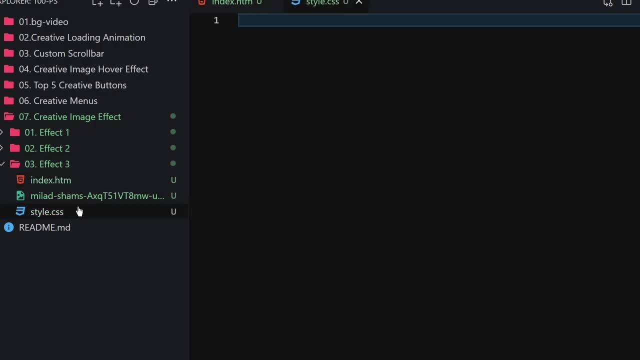 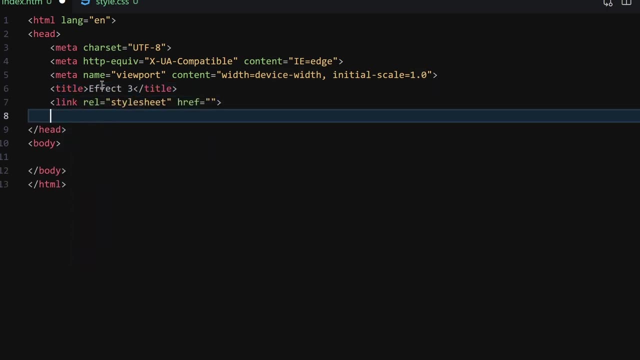 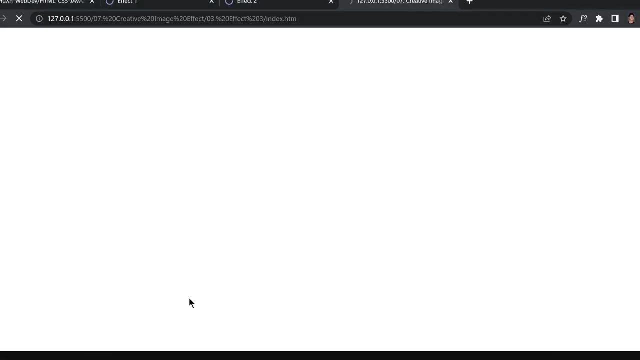 all right. so now jumping into our third effect. so i'll just close the other one. open my html and css, just write a doc type, html, effect. and number three, and then i'll link my css file to there. and now we are good to go. and now let's open that file inside a live server. and this one is going to. 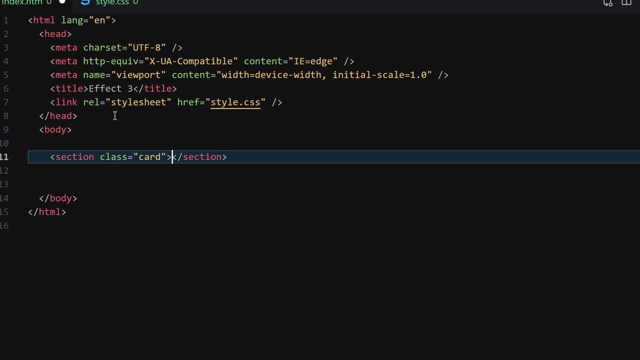 so for them we're going to have to write a section with a class of card, and inside this card section we have to provide image container first of all, and then we have to just specify our image. this is our image. now let's remove that all tag from there inside this section, or you know what not? 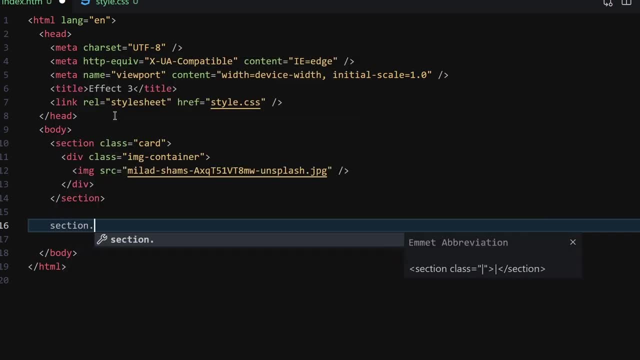 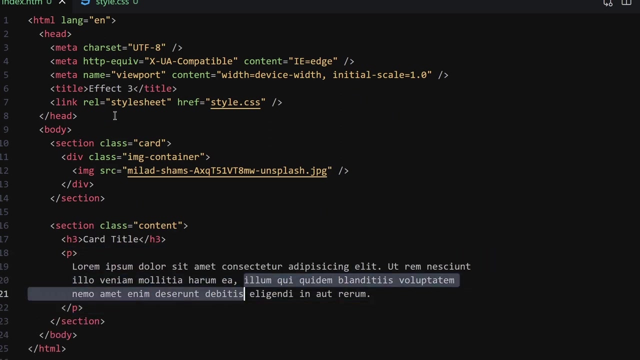 inside this section, but outside from that section we have to provide another section with the class of content, and inside this section we will just provide, like h3, h3 of car title, and then we have a graph of lorem, just how many you want. i'll just remove a few of them, like so, and then i'll just 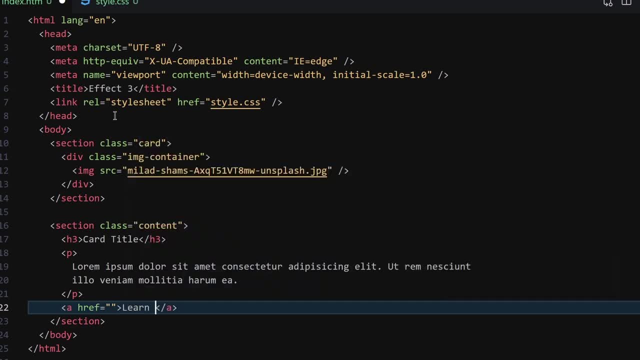 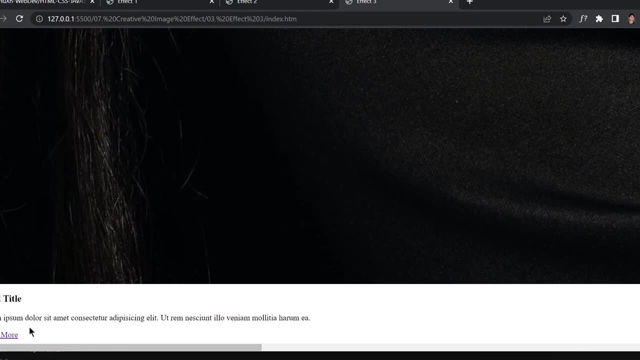 provide an anchor tag and it will go to nowhere except we will say, like: learn more, okay. so once we save our file, so this is our massive image and this is our card, this is our description and this is our button right here. okay, so, uh, now let's jump right into the css and style a little bit. 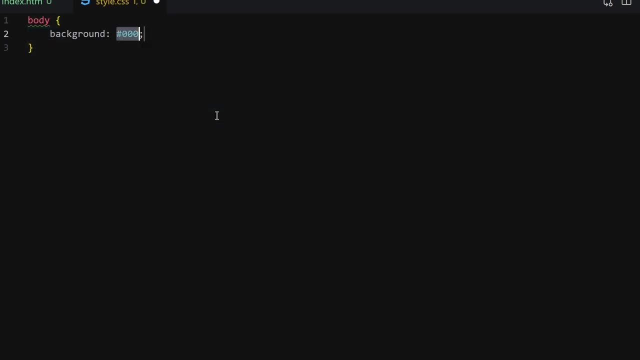 so let's start from the first one, which is a body. so background will be rgb, not a, but 23. copy it, paste it, paste it. and then height will be 100 vh, the same as the other one. display will be flex, justify corner will be center. align item will be center for family will. 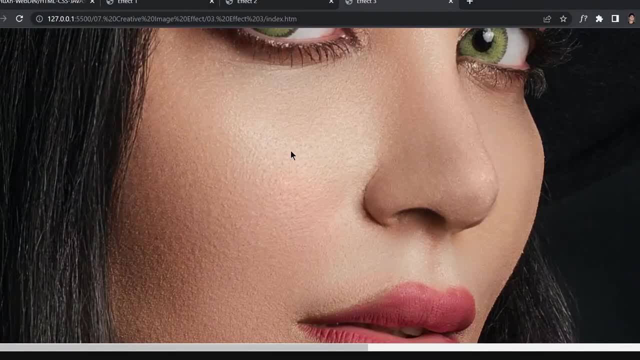 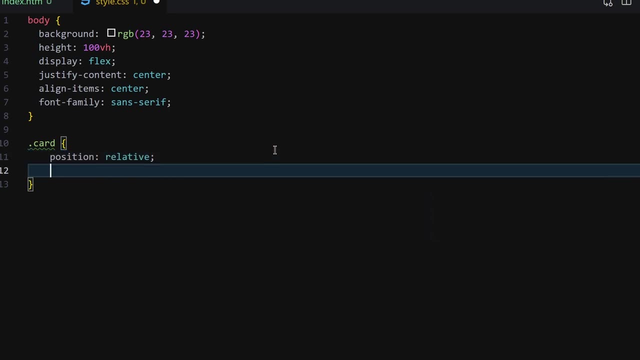 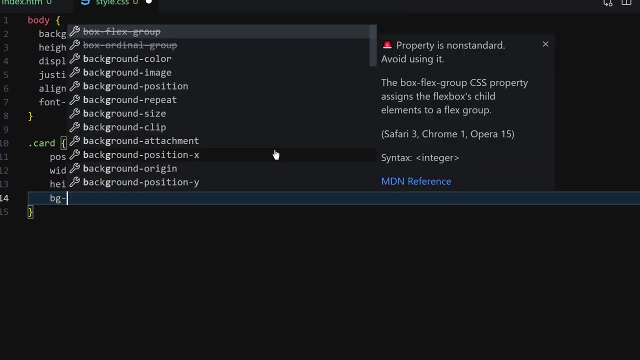 be sensor f and now save it. so everything is perfectly center, all right. so now let's select our card and then just provide a position of relative to it, and width will be 30 ram and height will be, in this case, 35. five frame, okay, and the background color will be just totally black. and then finally, box shadow. 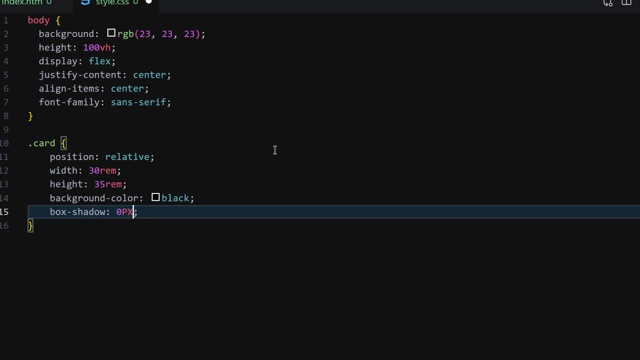 we're gonna have to put a box editor to it like zero pixel, and then 30 pixel, 30 pixel one more time, and then rgba: zero, zero, zero, zero, point five. okay, this will be our shadow, just a little bit, okay. so our images are really massive, so now let's make our image a little bit smaller inside that box. 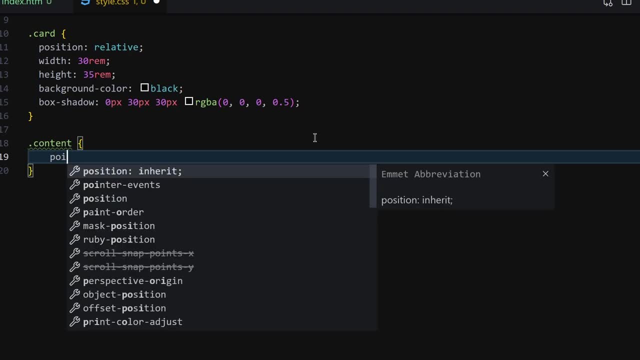 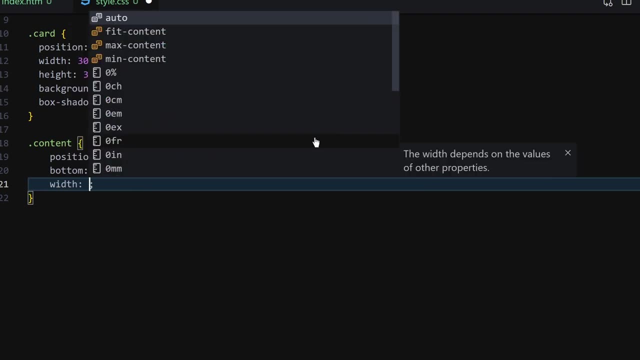 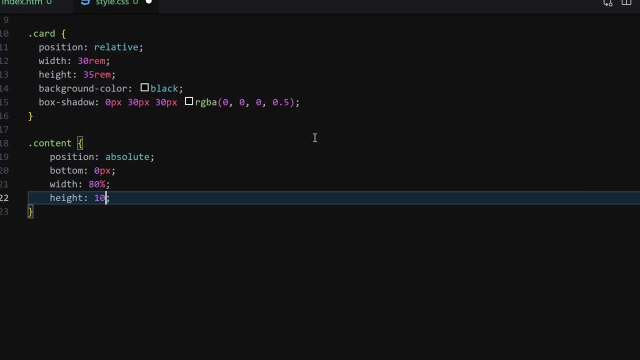 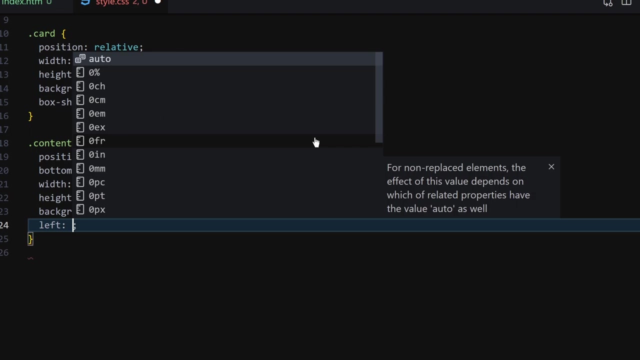 so now let's select our content and we have to provide a position of absolute turn and bottom will be zero pixel, and then width will be 80 percent- not percent, but pixel- yeah, it was percent, not pixel- and then height will be just 10 pixel and background color will be crimson and left will be just 10 percent and 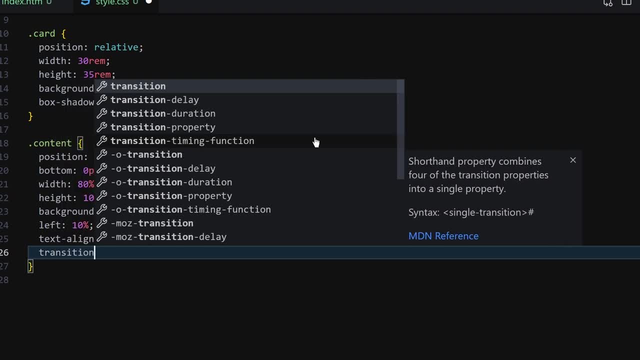 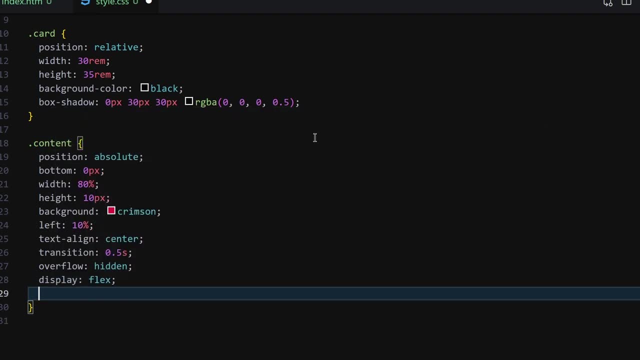 also, text online will be center and transition will be zero point five. second overflow will be hidden, as always, and display will be flex. now we are centering our content in center. a line item will be center. so now let's select our image and just make it a bit. 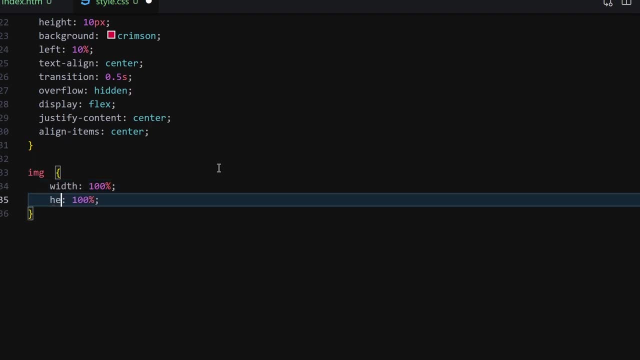 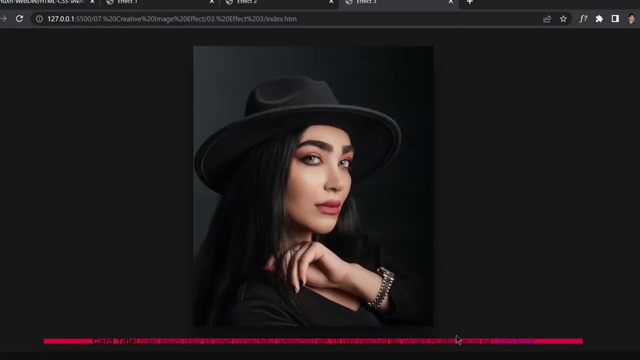 smaller, like width will be 100 and height will be also 100. object fit will be cover, not contents, but cover, and then we have a transition of one second. so once we save, it all right. so here's our image. is our content inside this image? so it's looking a bit weird, so i messed it up, so i'm gonna cut this. 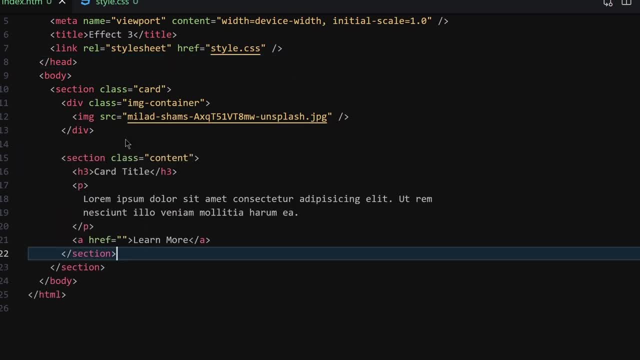 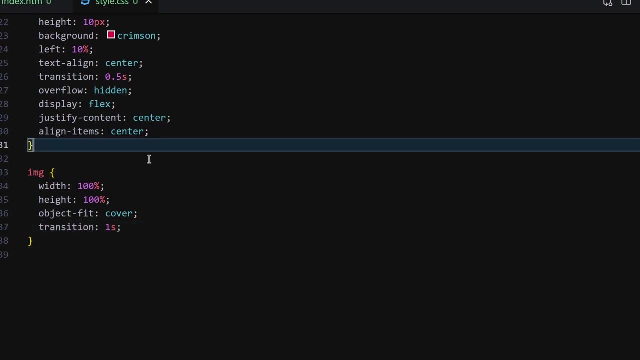 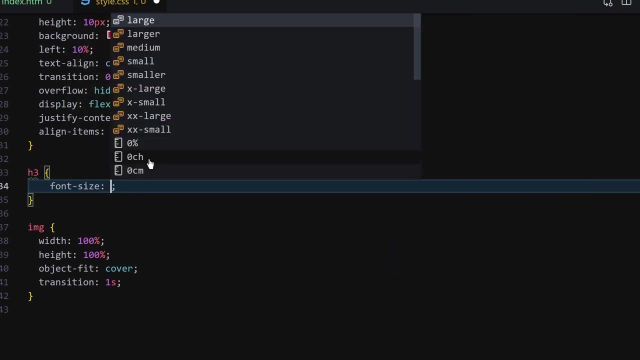 coding from there and paste it inside this section right here. so this is now looking good, okay, instead of just taking it outside. so now let's select order um h3 right now. so i'm gonna select my h3 and then just provide like font size of 30 pixel and text transform will be uppercase. now, yeah, 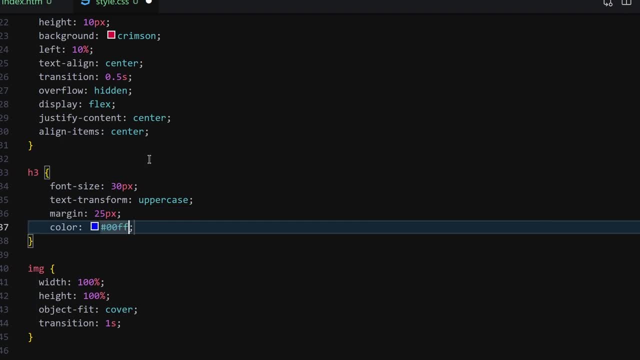 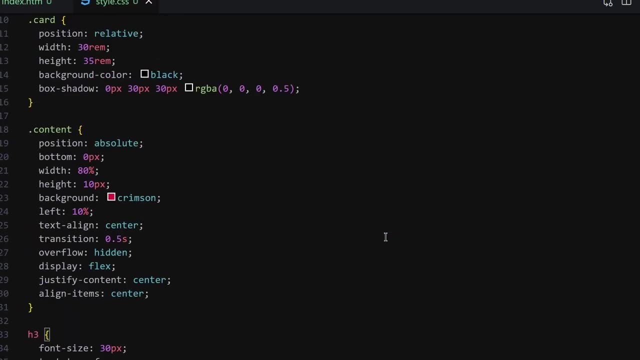 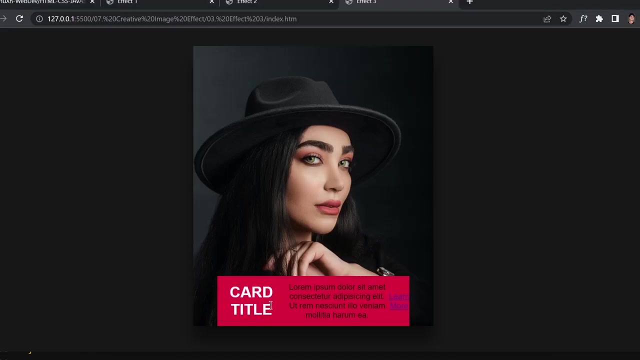 and margin will be 25. pixel color will be totally white. so once we save it, uh, we can't even see your content right now. so now let's give a little bit of height to it and instead of hunting 10, i'll just give him 100, so we can see our content right now. maybe 200 will be fine, we will just change. 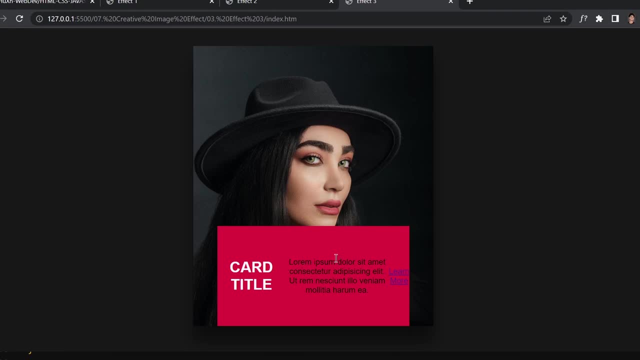 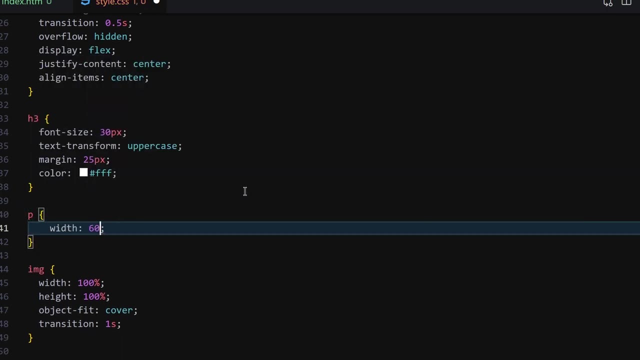 that in a second, but now let's first of all format all of them and then we can change it to 10.. all right, so this was h3. the next thing i'm going to select this paragraph and give a width of 80 margin will be 10 pixel, auto, and then. 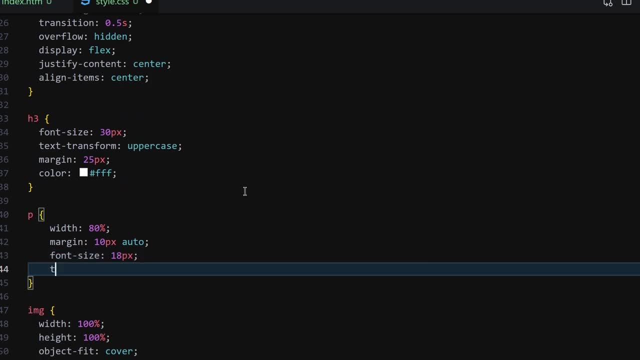 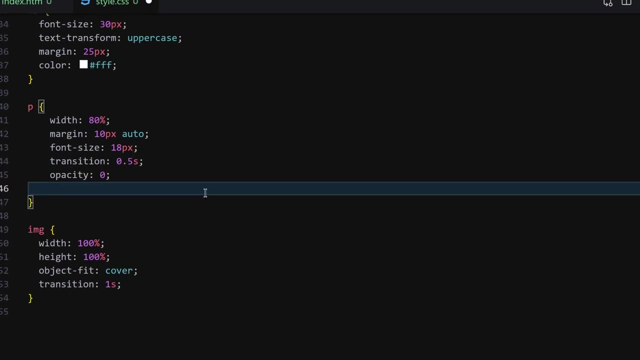 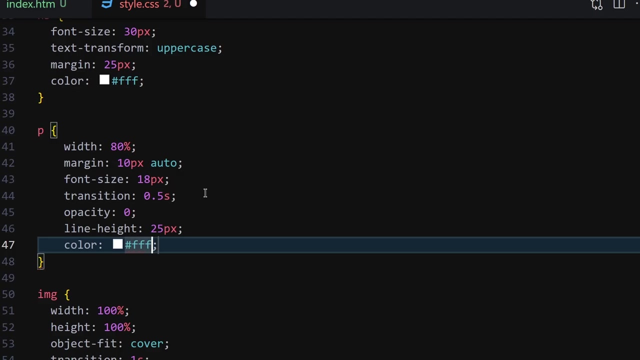 font size will be 18 pixel and then transition will be 0.5 seconds and then opacity will be 0, because we want to increase there whenever we have our or our mouse over thread, and then line height will be 25 pixel and color will be totally white. okay, so save it and this is our text, but let 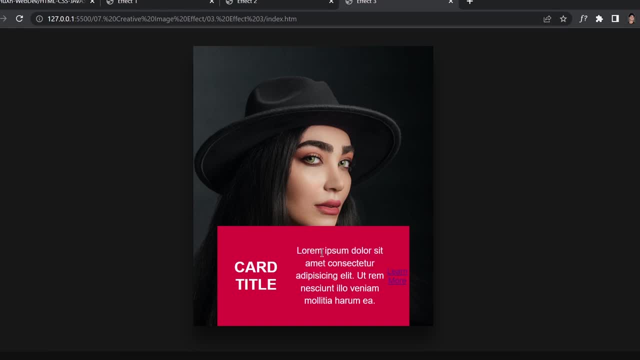 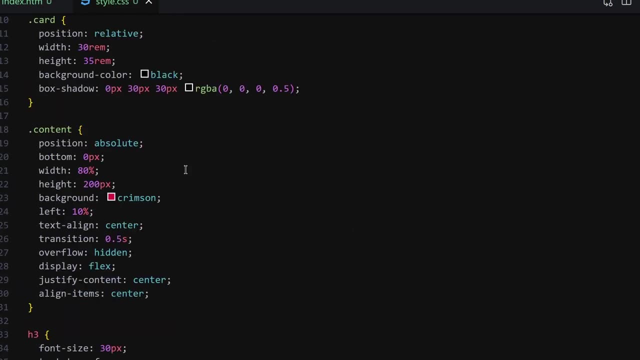 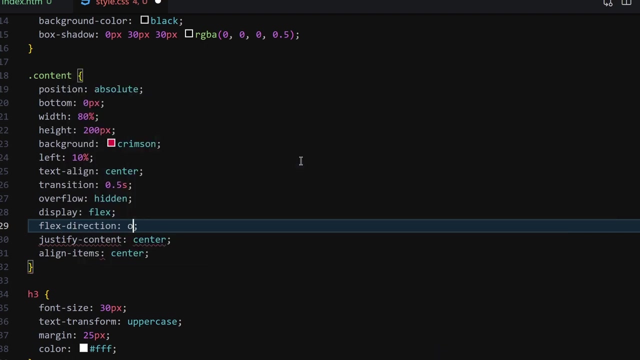 us go to opacity for now. and this is now our text. so now let's make it perfectly center. okay, i should have the poor display. um, where are you inside a content? where is our flex box? okay, so here i will just add like flex direction column, so save it, and now it's looking a bit cool. so now let's format. 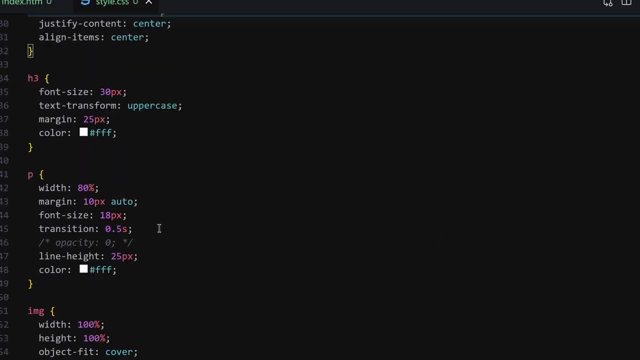 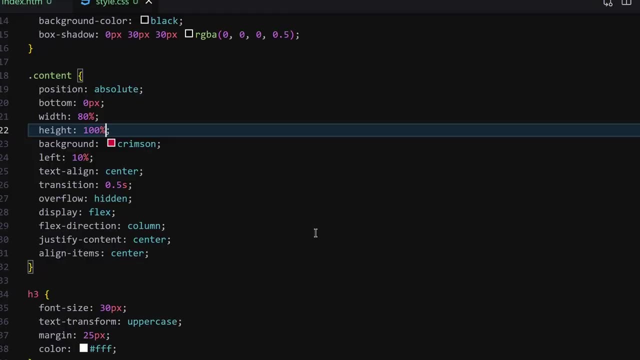 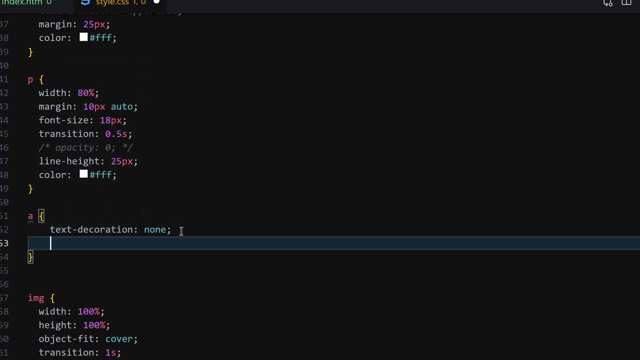 this button very quickly. so here now i'm gonna just do is: it will be also 100 from now, because everything, and now let's format this button. so i'll just select that button really quickly. so i'll just select that anchor tag. inside this anchor tag, text declaration will be none. uh. 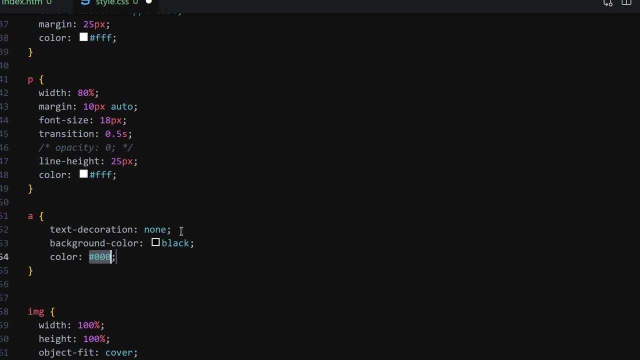 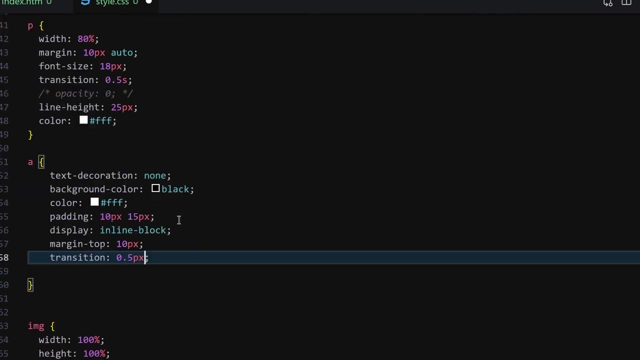 background color will be black and then color will be, uh, totally white, and then a padding will be 10 pixel and 15 pixel, and then display will be inline block, okay, and then margin top will be just like 10 pixel, and then transition will be 0.5 pixel, not pixel, but just a second, and then opacity will 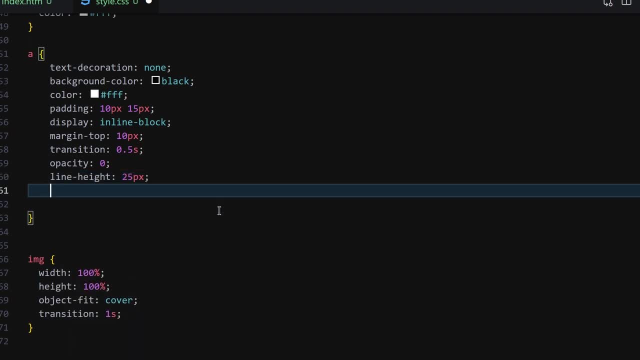 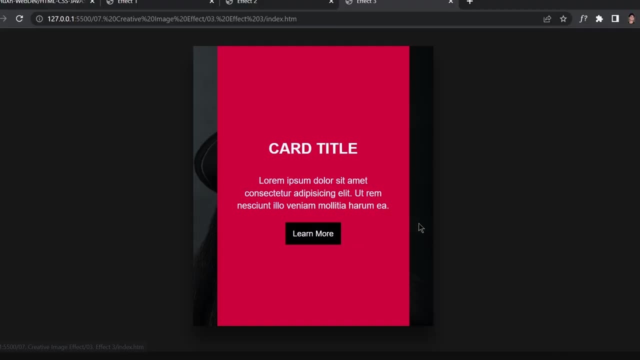 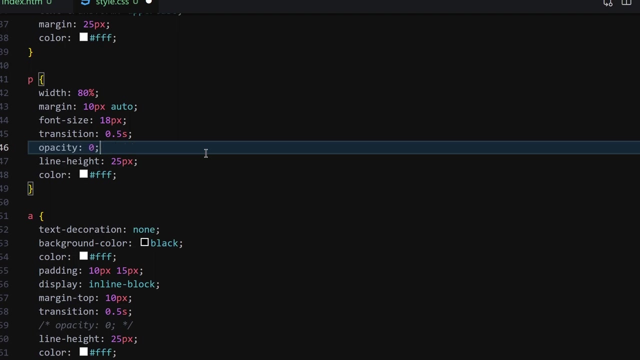 be also 0 and line height will be 25. pixel color: a bit totally white, and let me comment this. opacity 7 and this is how our button will look like. okay, so now it's looking a bit cool, all right, so now let's add our hover effects here. so i'll just uncomment this opacity and also uncomment this. 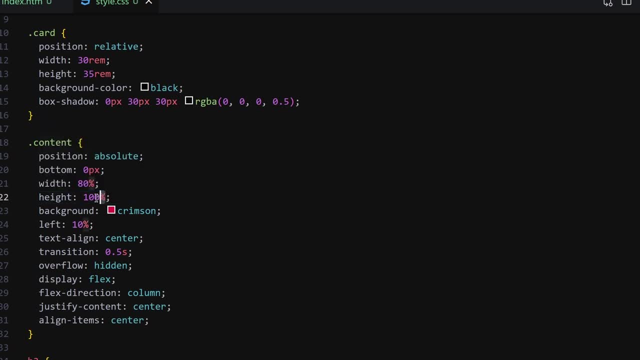 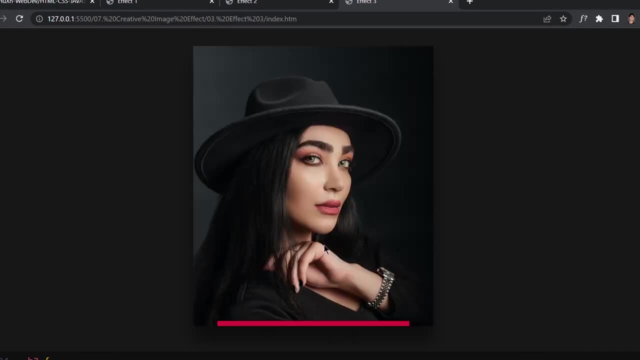 opacity as well. so i'll just uncomment this opacity and also uncomment this opacity as well, and now let's change this to just like: uh, 10 pixel, again, save it and this is how it looks like right now. okay, so our content is not showing. nothing is showing because we just provide the. 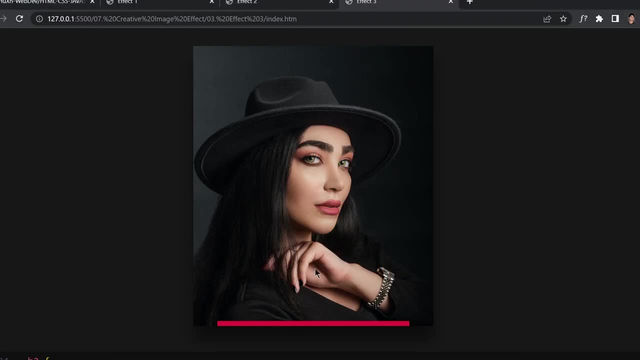 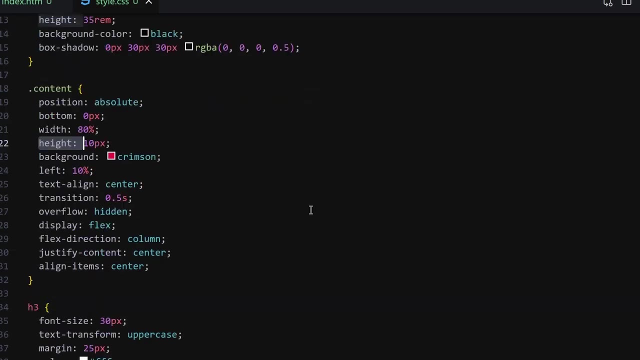 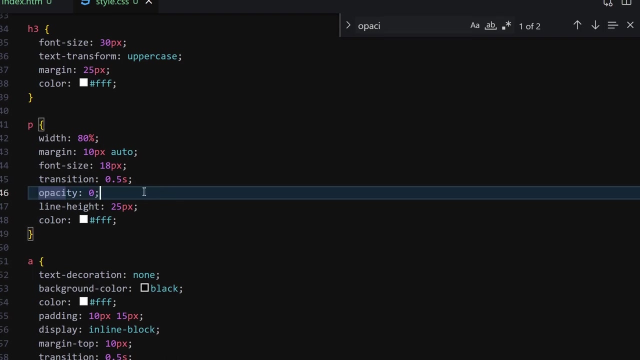 height of 10 pixel. so whenever we hover over through this uh card, so it will take the entire space, like width will be 100 and height will be 100 and opacity will be just set to one, so it will just show up. that's why we provide these opacities like uh. where are you opacity? so here? 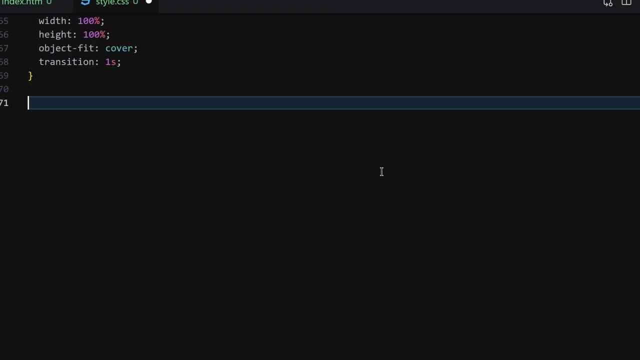 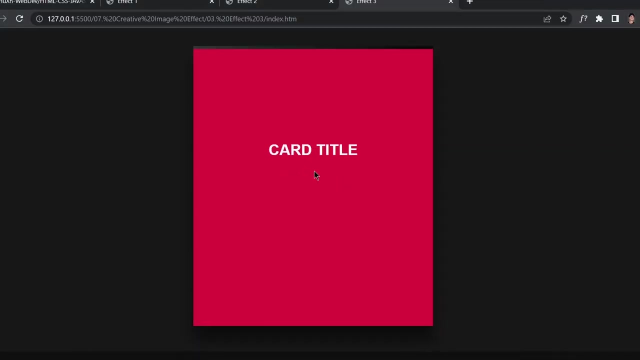 is the opacity, and here is also the opacity. so now let's change that. so whenever we hover over through this card content, so we want the height to be 100 percent, we also want the width to be 100 percent. we want the left percent to be zero percent. so whenever we hover our mouse over to it, so here. 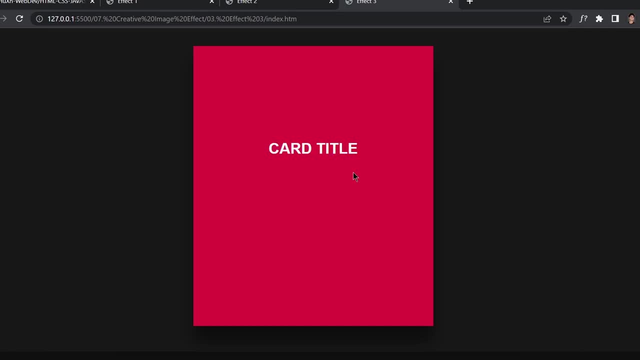 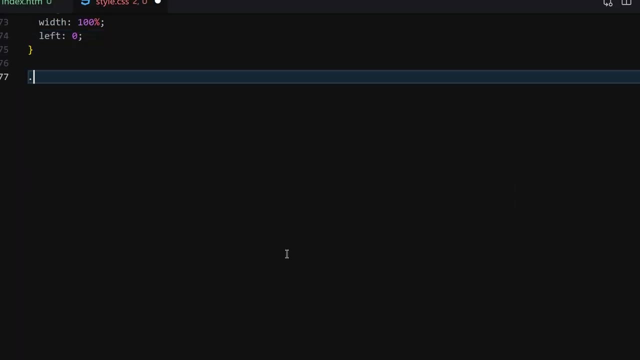 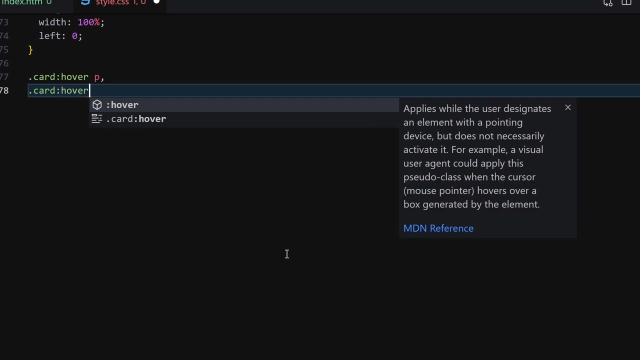 you can see, the card will take its totally place and we cannot see the order counter because we just provide the opacity of zero. so now let's change that to like something else. maybe, uh, i don't know- will be hover uh. now let's select our paragraph comma. let's also select our hover uh anchor text. 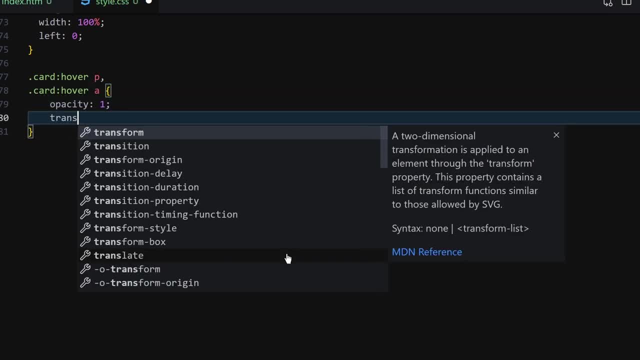 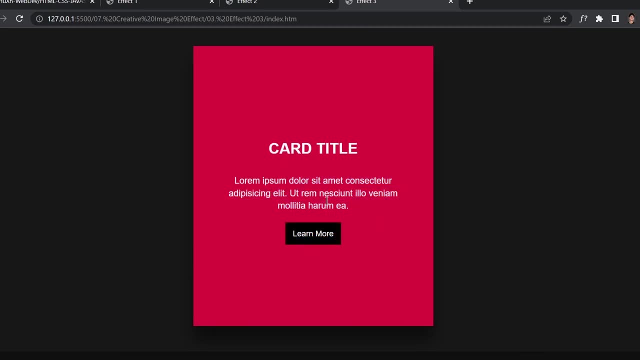 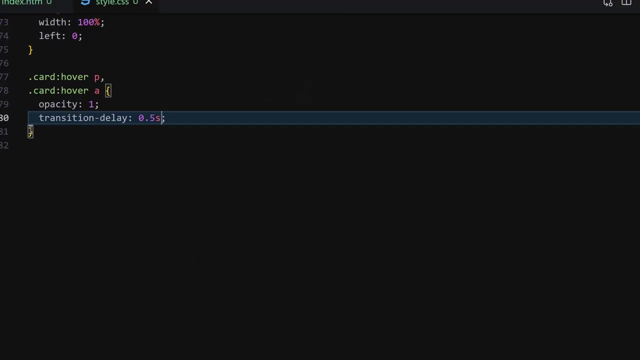 so um, opacity will be one and transition delay will just take a bit of time, like 0.5 seconds. so now, once we have our mouse over to it and so here now you can see, our content is back. so it's taking a bit of time, but that's cool. that's why i provide this transition delay to her. 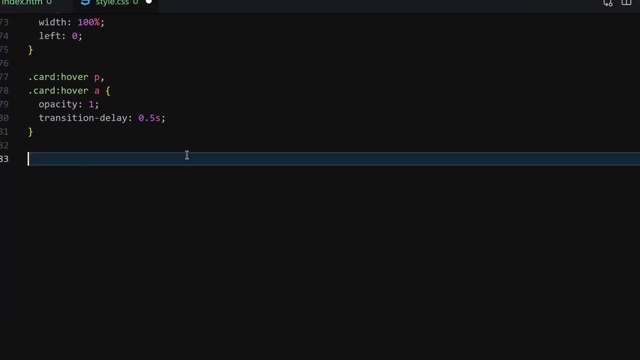 and now let's select this image container. so what i'm going to do, i'll just write image container and then just provide a position of absolute: top will be 0, left will be 0, width will be 100, because we want this image to take this entire place, and height will be also there. and then 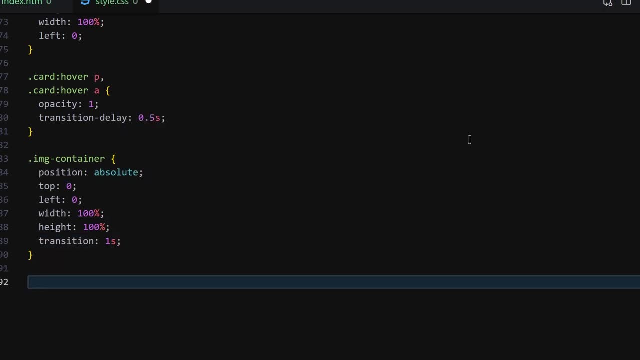 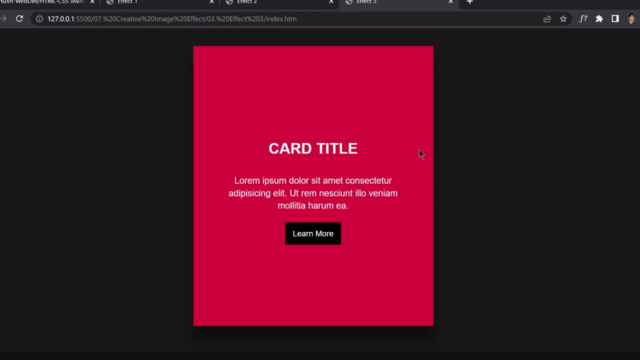 transition and one second. okay, so now our image is looking like that, but if we hover our mouse over to it, like our hover image. so once we hold our mouse over that image, so the opacity will be zero. okay, so now let's do that. all right, so that image will be gone. here you can see the opacity like: 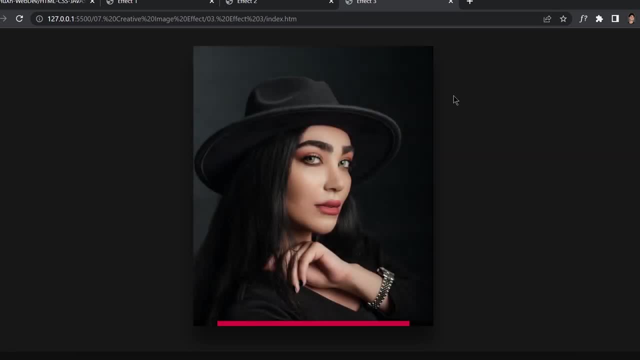 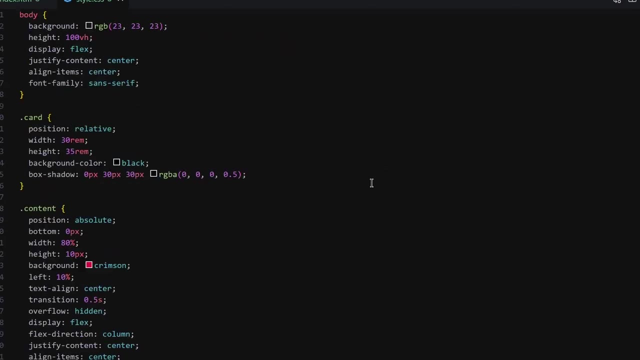 just focus on this image. it's just like decreasing the opacity is just becoming zero percent. this card is taking this place. okay, so that was quite simple and easy. i talk a lot. oh my god, i can't even speak no more. all right, so now let me review all of the code, not all of the projects. 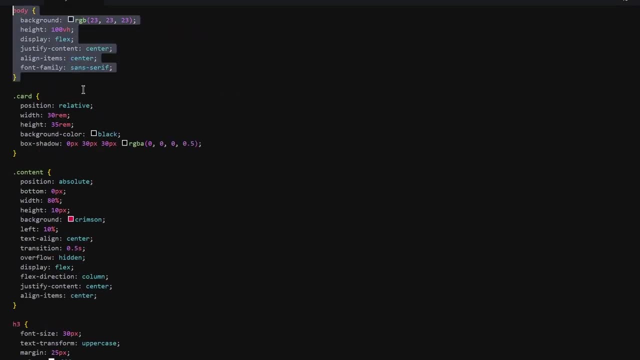 but just this code. okay, all right. so the first thing we do is we just set everything and we provide our height period of hundred vh, and then we create our card and we provide a position relative to it. we give a width of 30 and height of 35. bag weapon color is totally black and box shadow. we just 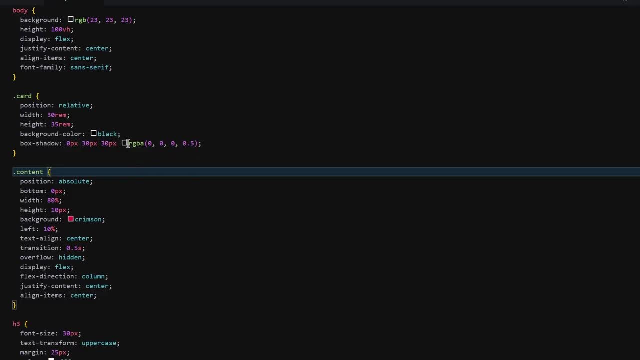 provide this a little bit of box shadow. here you can see that if i change the color of it to like, uh, i don't know, do maybe and here you can see that box shadow right now. so let me just change that to there. so here you can see, we just provide that box shadow along it. all right, okay, now that. one is stopped here. so i've got a whole bunch of enfants item and i've undone a bunch more of of them right and now you guys can see we have a physical step by step of adding no color to that. pretty clear, like this view: okay, a problem, i'm always buying this little non- impresionable. 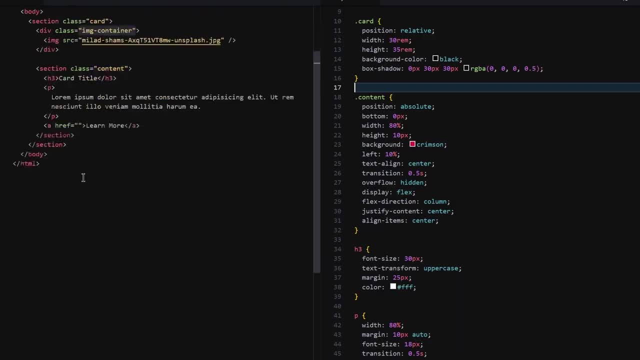 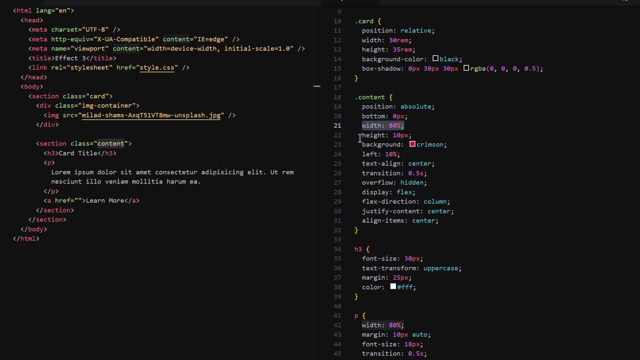 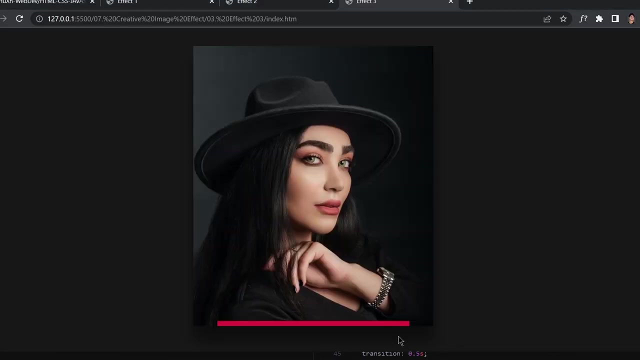 shadow. then we have our content container like this content: where are you? this content right here. so this content is position absolute. bottom is zero percent. width will be 100 percent. height will be uh, 10, 10 pixel, because we just want them to be look like this. so whenever we have our mouse, 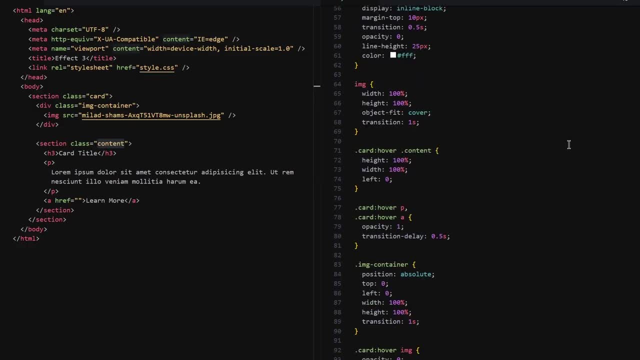 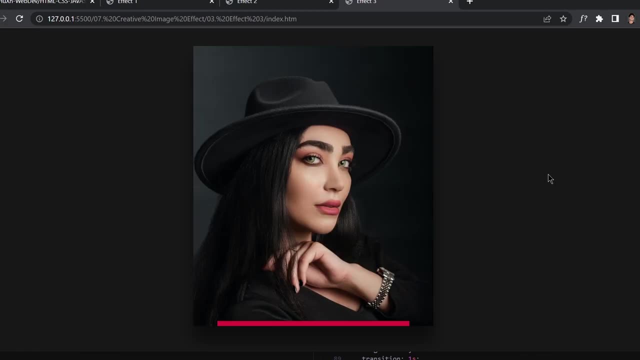 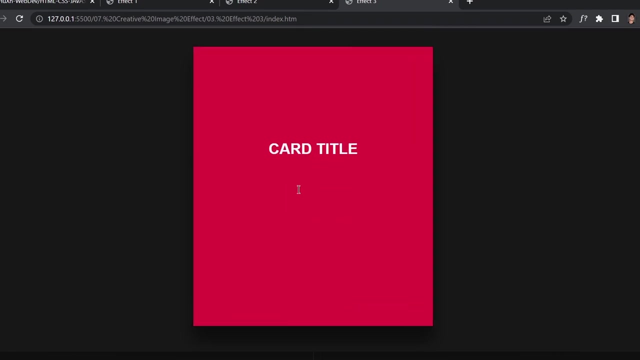 ordered. so this code will happen. where are you? so this uh code will happen. so whenever we hover on mouse, ordered. so the height will be 100 and the width will be also 100, so like this: okay, and then we pour the transition delay to it. so this text will take a little bit of time. so this text. 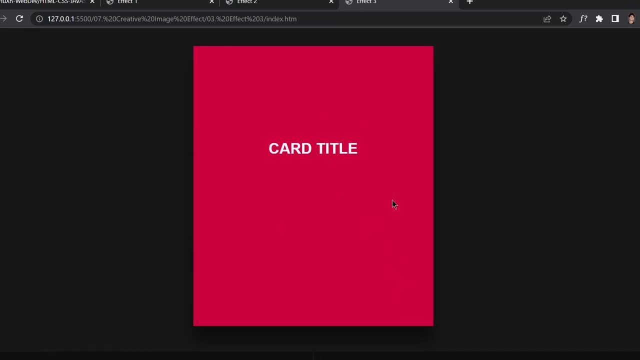 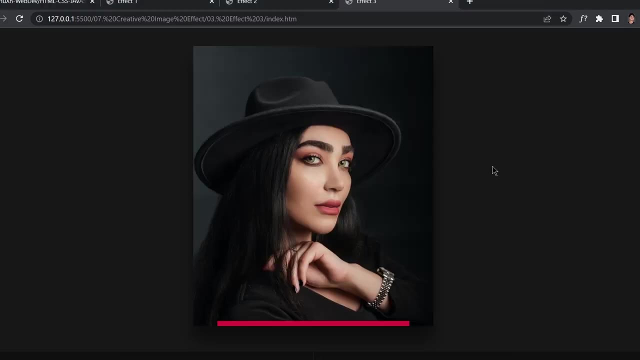 will take a little bit of time, and so is this button. so focus on this area and this. what's going on anyhow, then we just check our container. so whenever we hold our mouse, altered so that container, that image will be just uh, gone. that's because of this opacity right here. 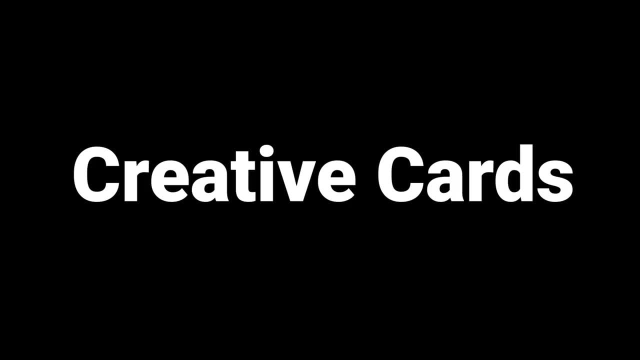 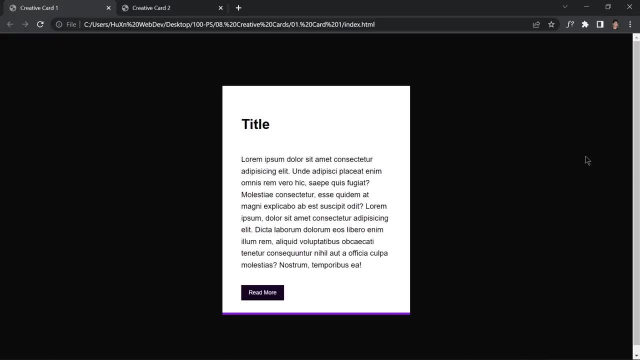 and will take one second to happen. again, susan, and welcome to the ad project of this course. so in this video, we are going to be creating a cards animation by just using html and css. so now the first card which you're going to be creating is once we have our mouse altered, so this container will take its entire space and 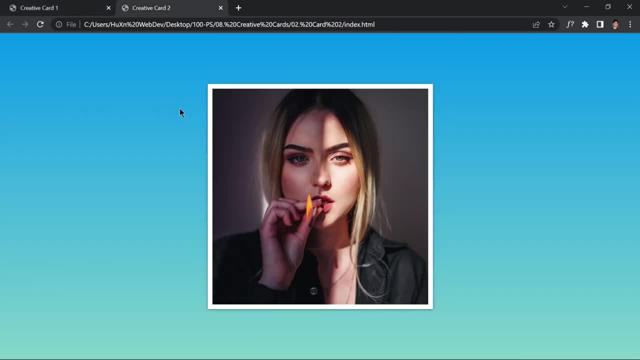 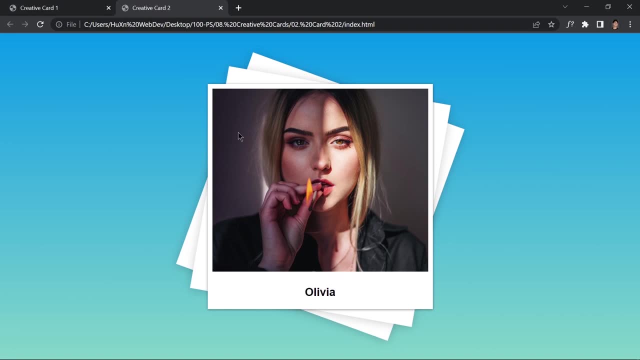 if you leave so, it will just decrease. so the second creative card which you're going to be creating is once we have our mouse over to this picture. so we are going to be using before and after selector, so we would get this kind of animation and also these, um, these background container right here. 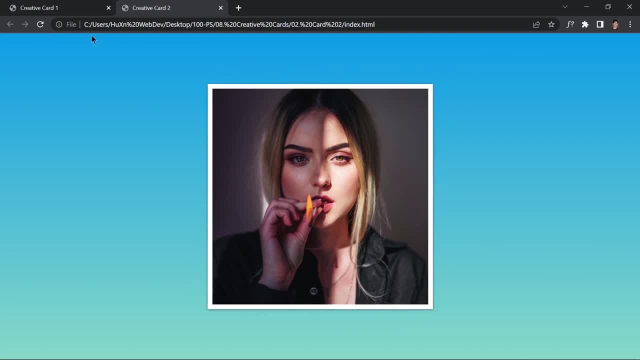 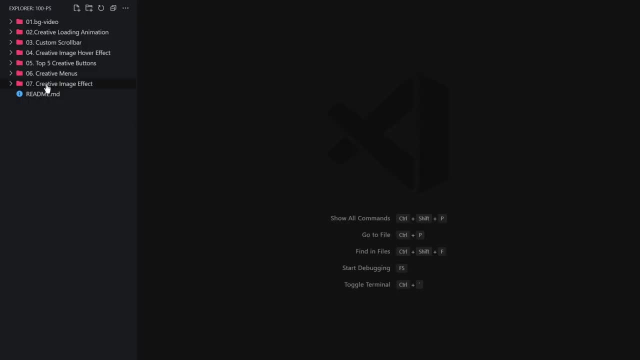 like background cards. all right, so this is we are going to be building in this video. so, without wasting any time and now let's jump into our code editor and write our code in the previous, where we've created this uh image effect. in this video, we are going to be creating a cards by just using 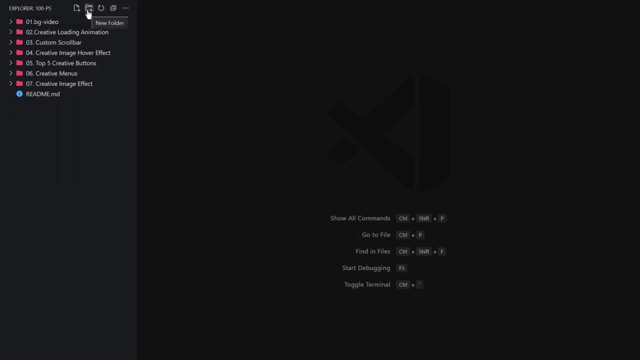 html and css, not javascript. no css preprocessors like sas, etc. so i'll just give a name of like 08 creative cards. okay, so then i'm going to just write two folders, card one, or just a one of card one, and then oh, two of car two, not cartoon, but card two. then i'll create a file, indexhtml. create new file. 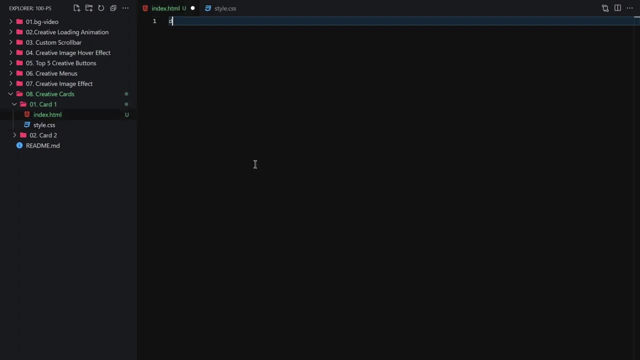 stylecss. then i'll just write my doc type html in it. and now here i'll just change that to like: uh, create creative card. um, one will be fine. then i'll link it with my css file and now i'll just cut both of them. copy both. 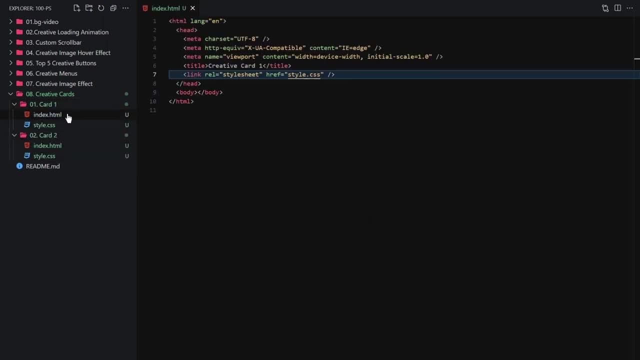 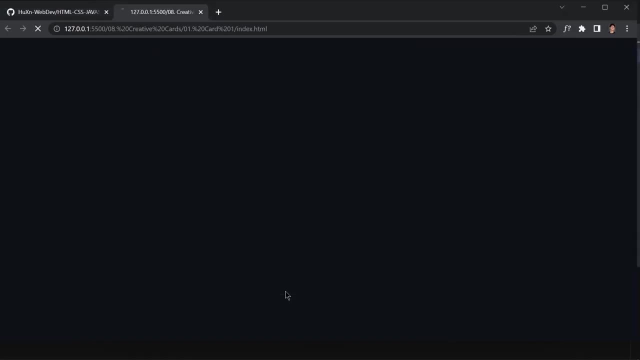 of them and paste it inside this project as well. so now let's start from the first one. zoom in number so that you guys can see everything a bit better. and now let's right click on and go with the live server. okay, so for html. you're not going to be writing crazy. 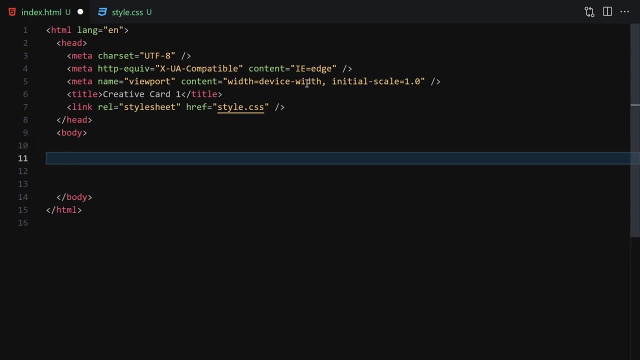 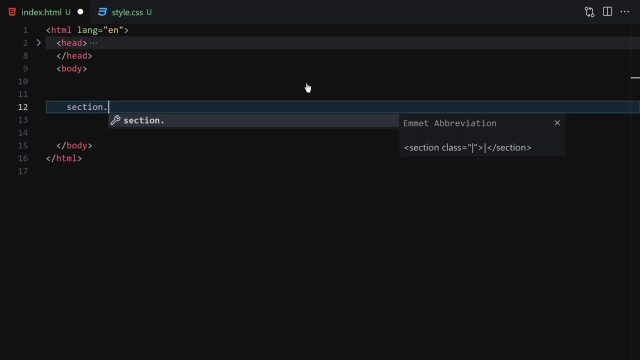 html, but we are going to be just writing a simple amount of html. so the first thing is i'll just close. that matters. from now and now, section will be card container, okay, and then we are going to be writing article, the class of content inside this content. we are going. 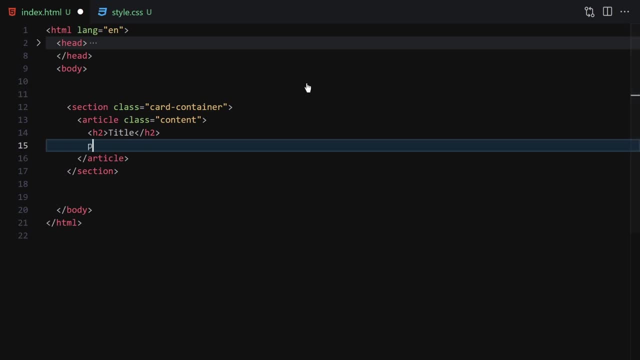 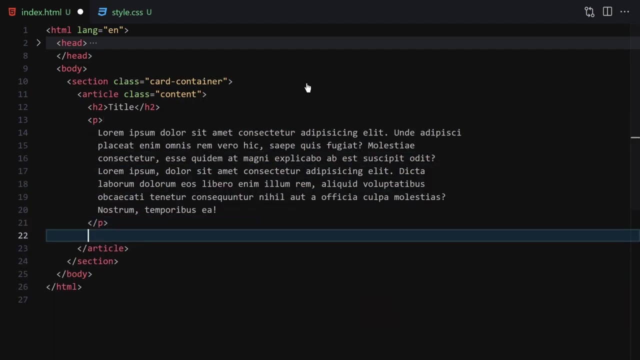 to be writing h2, which is the set title, and then we have a paragraph. so i'll just write lorem one time and hit tab, then, uh, lorem one more time, i hit tab, so it really gives us double lorem right here, and then i'll just provide an anchor tag which will go to nowhere. 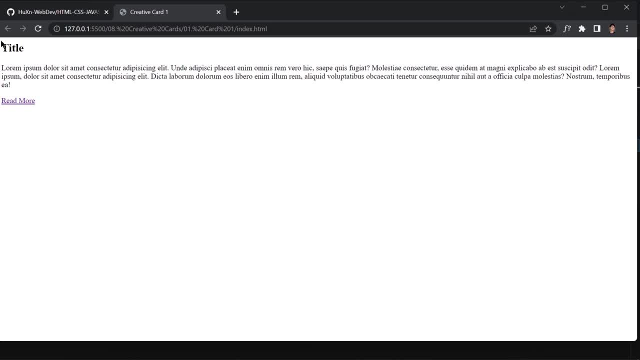 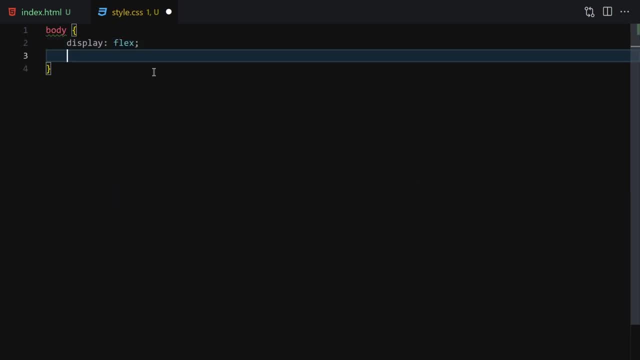 and read more and save our file. and here is the result of our html code. okay, so now let's begin tour styling. so i'll just write a body display with flex, because we want everything to be perfectly centered. so that's why we are using a flexbox and we will just give them a form: family. 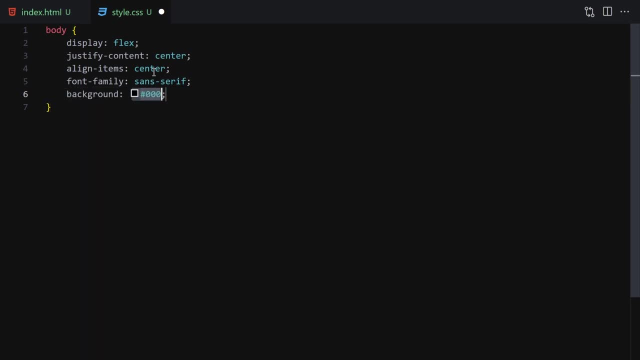 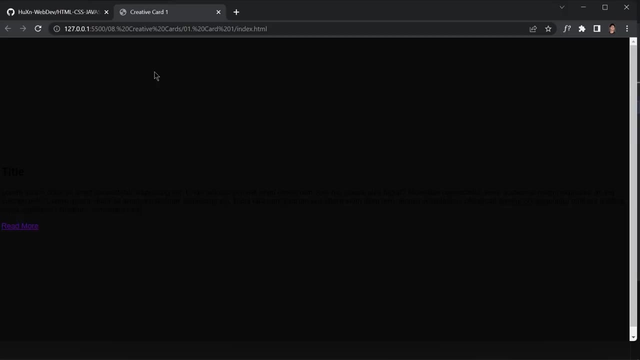 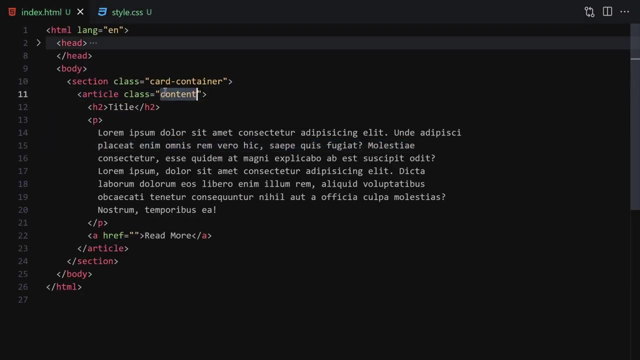 of sensor. you can choose whichever form you like, and then background color will be just rgb, and then 10 comma 10 comma 10, and then height will be 100 bh, and once we save our file, so we cannot see anything, but everything is perfectly centered, okay. so now let's begin styling this content. 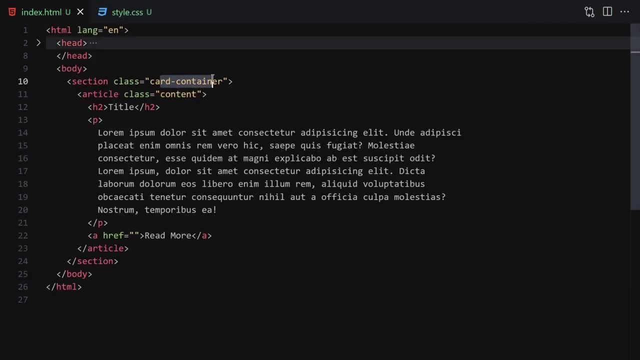 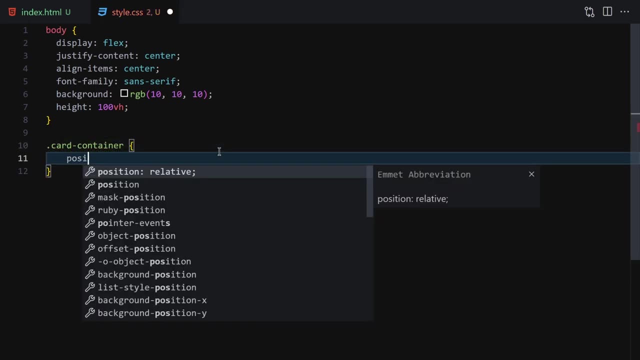 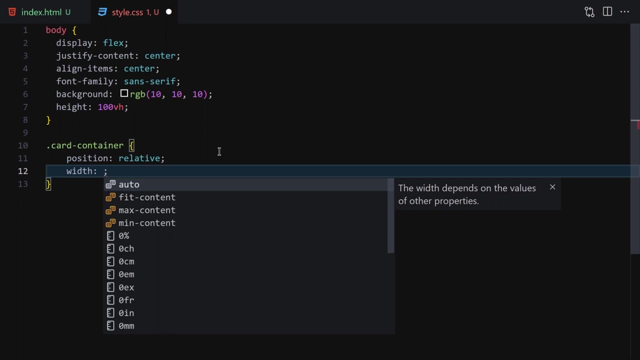 container, or, uh, i mean like this card container right now. so i'll just write like card and then container. okay, so inside this card container i'll just write position to relative, because you want the other stuff to be position absolute. so this one will be position relative and the width will. 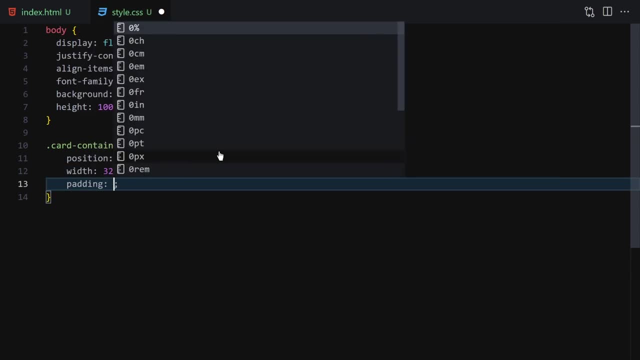 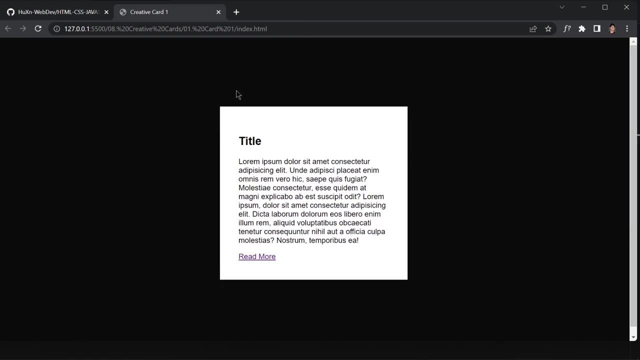 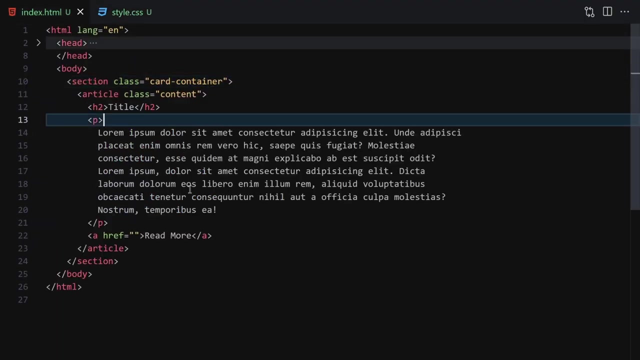 be 320 pixel and the padding will be just 40 pixel padding and background color will be totally white and then overflow will be hidden and once we save it, and this is our card right here. okay, so now we have our first card and now we want this other content to take its place. so let me show you. 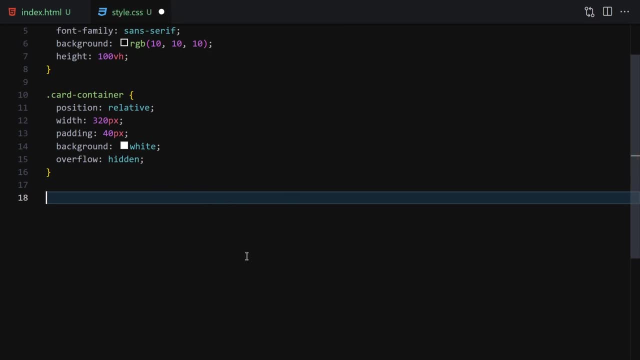 that just in a second. so for that we have to use um before selector. so i just write like card container and then before, and then content will be just empty content, we don't have to provide anything to it, and position will be absolute. because this is position relative and we want. 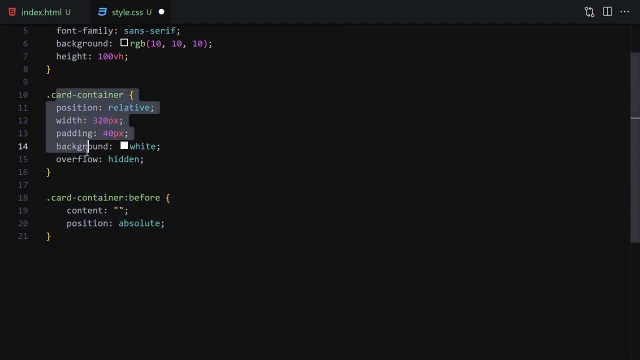 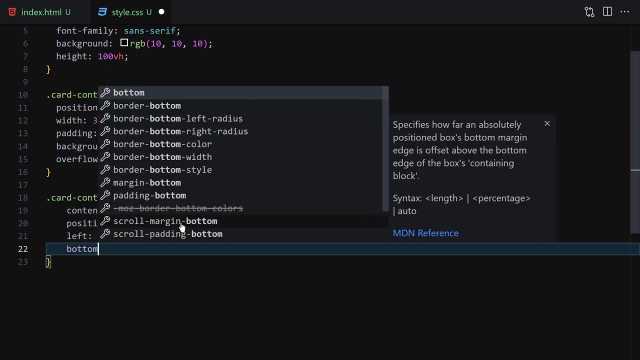 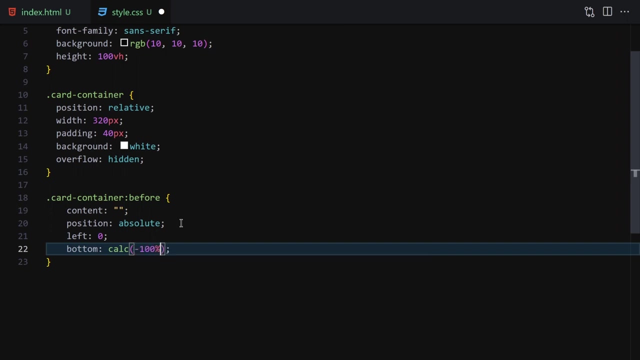 absolute, because we want this before to be inside of this card container. okay, so position: uh, absolute, then left will be zero and then bottom. we are going to be using something called calc which allows us to do calculation, and then i want to just use like minus hundred percent plus five. 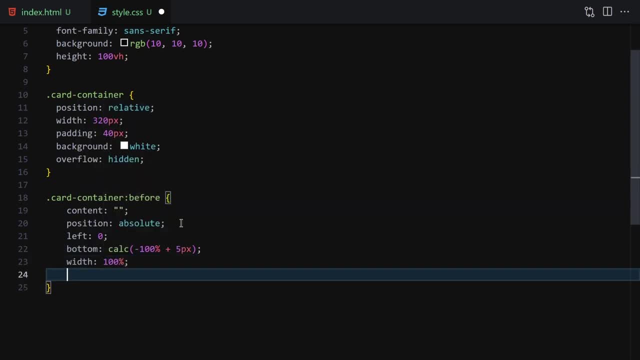 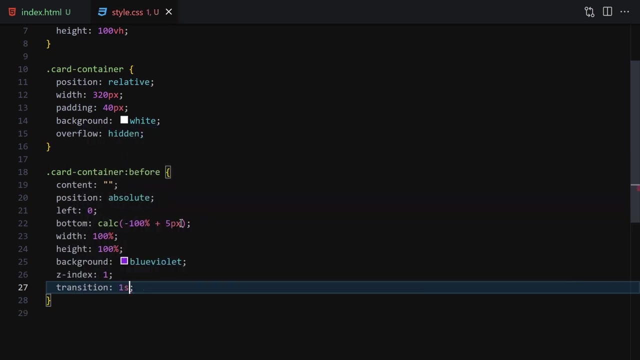 pixel, okay, and then width will be 100, and then um height will be also 100, okay, and then we have a background color of blue- uh, what was that? blue, violet, or whatever you want to call it. and then z index will be one- uh, just minus one. no, not minus one, but just one. and then transition will be one second, because we will have 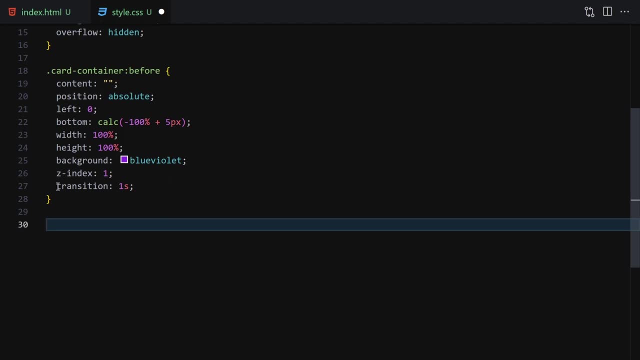 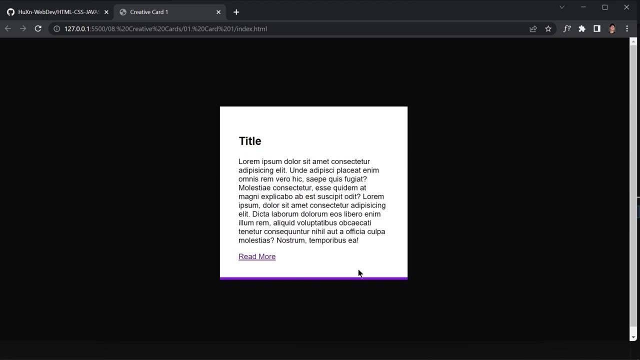 a hover effect for this um before selector. so that's why we are providing a transition to happen smoothly. okay, so once we sell a file. so here you can see, we have this like border bottom right here, because we have a width right here and we also have a height, but we don't. 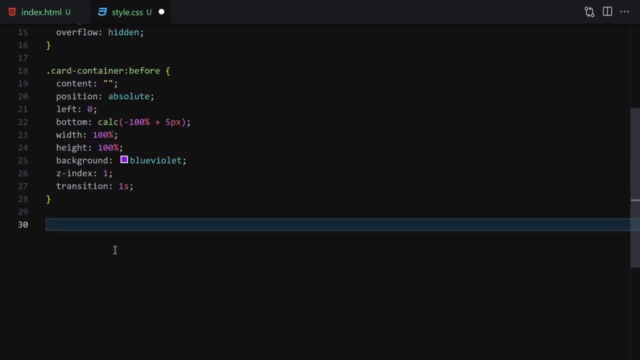 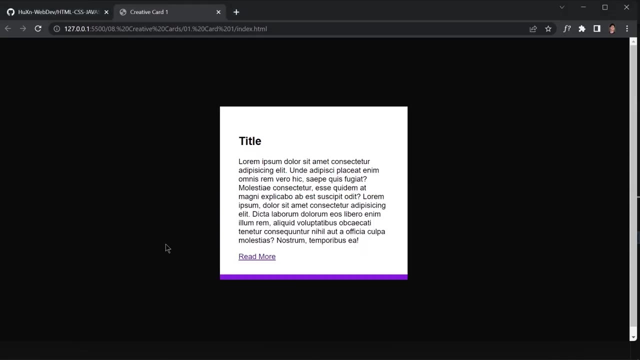 provide any hover effect. so we're going to have a higher, but we're going to provide any hover effect to it. so now let's provide a hover effect to that like car container. once we hover over to the before selector, then we have to just provide the bottom to zero. so now, here you can see whenever we hover. 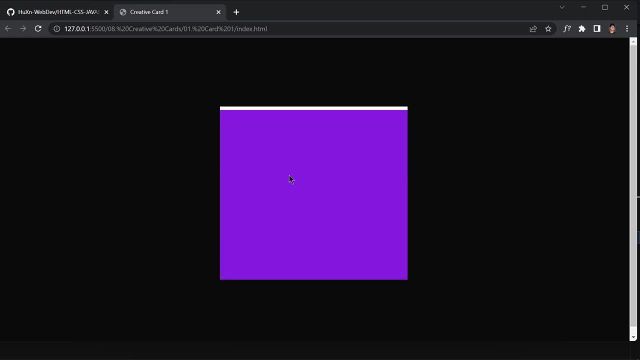 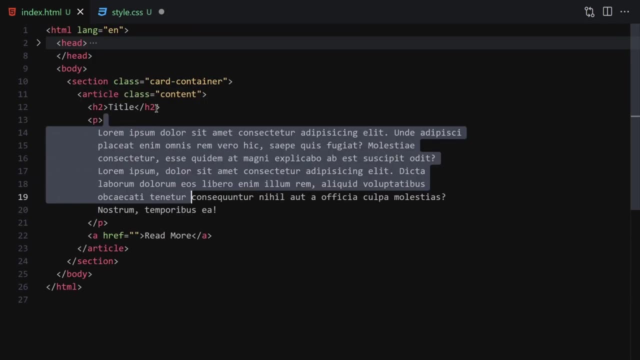 our mouse over to it, so it will take the entire space right here. okay, so this is what's happening behind the scenes. all right, so that was the first one. so now let's style our content right here, this content container right here. so now let's just style that a bit. so then i'm gonna have to select. 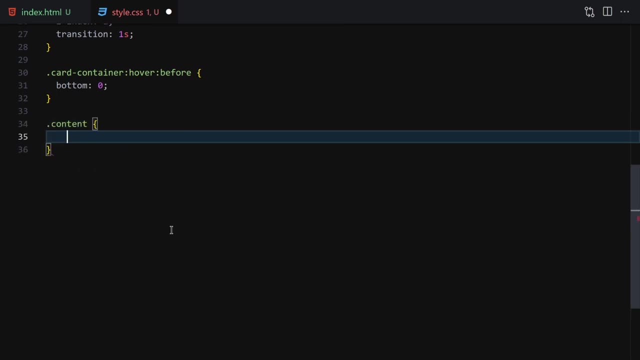 that content. so i'll just select the content. so i'm going to select the content. so i'll just select this: like content inside this content. position will be relative. like outside of that container, color will be totally black, z index will be, in this case, two. the other one was one, so this one. 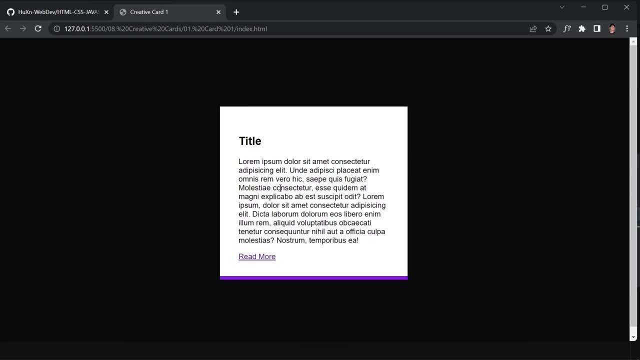 will be two and then transition will be one second, because for that we want to provide um, the what way? before that, we are going to be using a hover effect, and here you can also see, like whenever we have our mouse ordered. so here you can see the text is appearing. so if i just remove all of them, 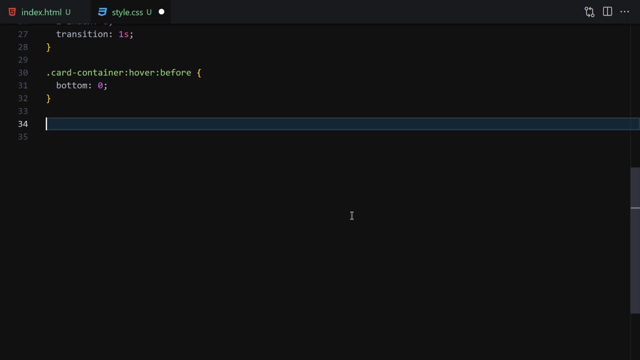 save it. and now, here you can see, all of the pages are going to be in the same position. and then here you can also see, like when are we? our mouse altered? so here you can see the text is appearing. so, if i can see, the text is now shown, and if we just undo it and save it, and here you can see the text is, 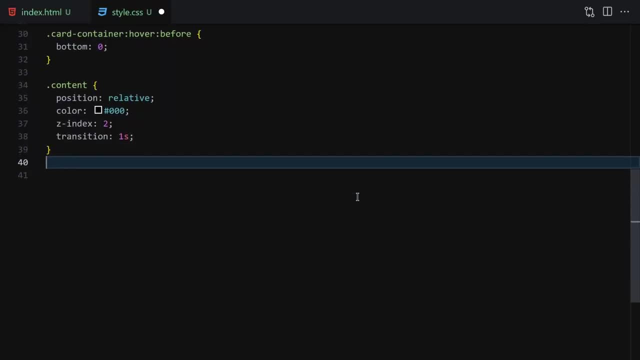 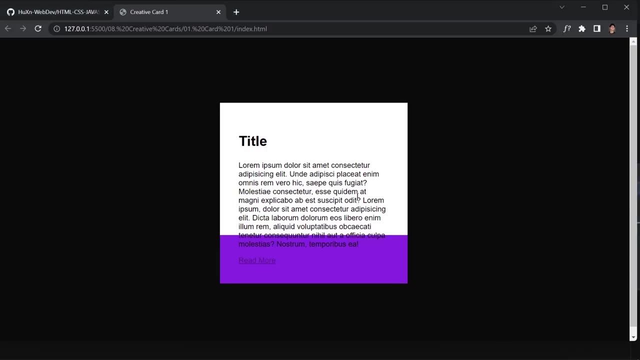 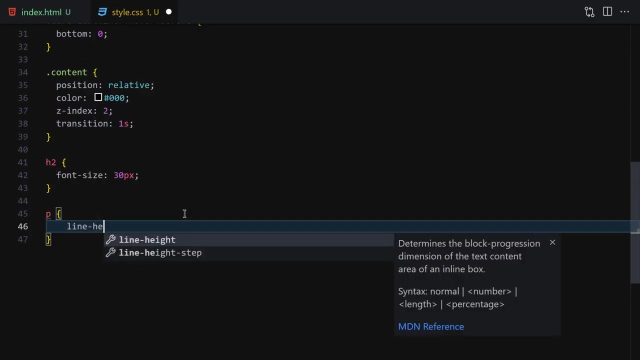 now here, uh, all right. so now let's select our h2 very quickly, and now let's format it like: font size will be 30 pixel, um yep. and save our file. so here you can see, the h2 is a little bit bigger right now. and now let's select our paragraph, and line height will be 25 pixel, and then we have like: 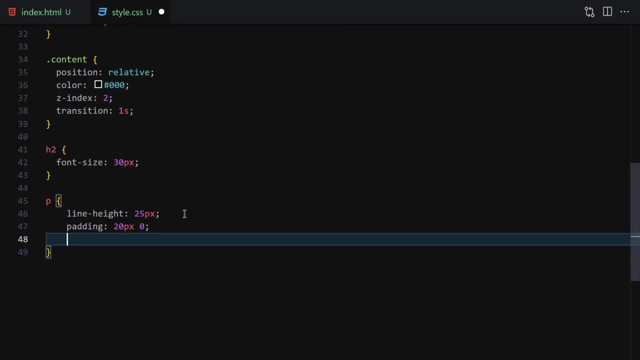 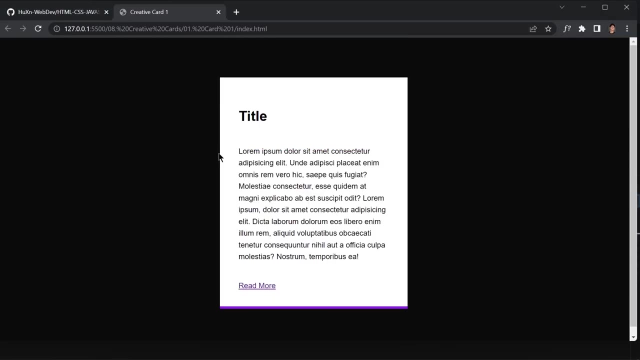 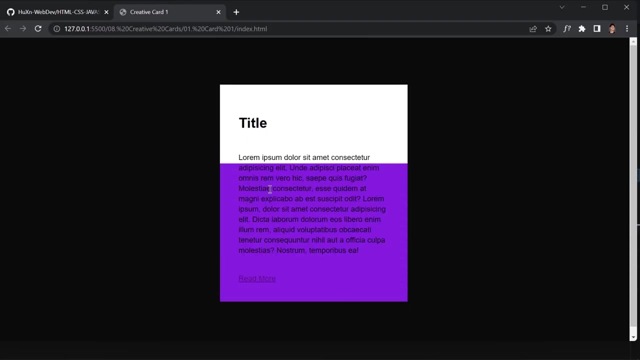 a padding will be 20 pixel and 0: 20 pixel from top and bottom and 0 for left and right. margin will be also 20 pixel from top and bottom and 0 for left and right, and here you can see we have this a little bit space right here, okay, so, uh, we can just, i guess i'll go to 22. this is looking a. 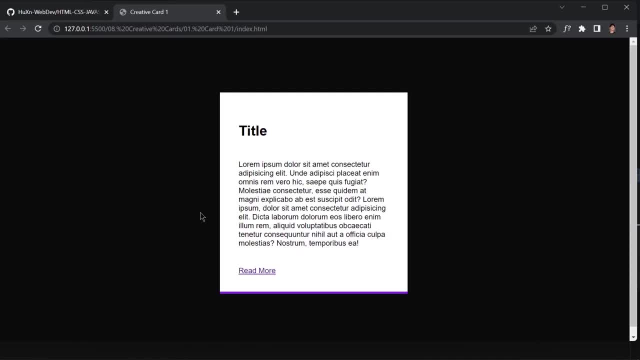 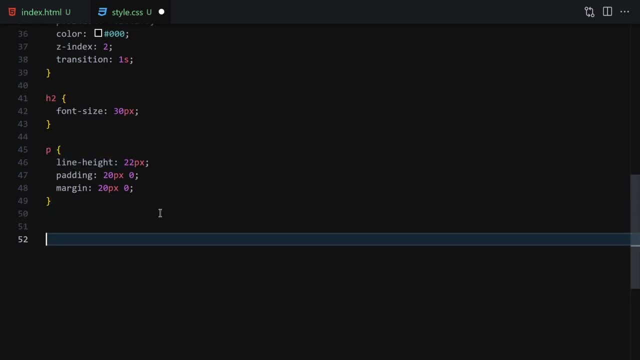 bit cool, uh, if i don't provide any line height to it, so it's looking a bit ugly. yeah, i guess that would be fine, all right, so this was about the paragraphs, and now let's format or anchor tag this one right here. so for that we're going to have to just select it. 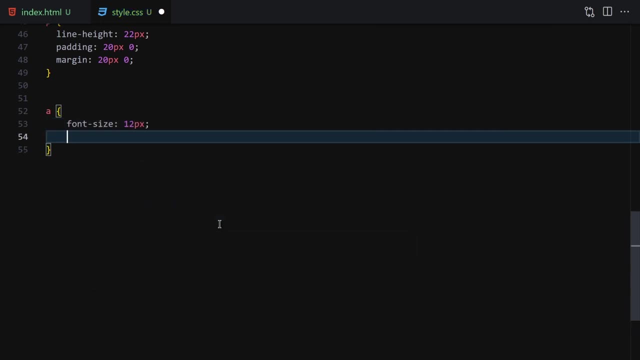 and font size will be 12 pixel and then color will be totally white and text decoration will be none. and then we have a background color of rgb 22, comma 7, comma 7, and then we have 35. all right, so this is our color. then we can provide padding of 0.6 ram from top and bottom. 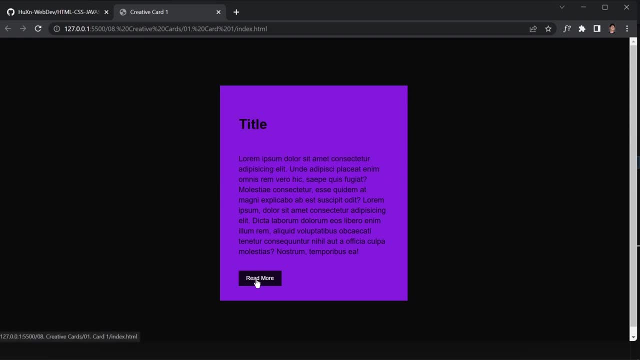 and for left and right rim. okay, so this is our button right now. and now. what else do you have to do? because whenever we hover our mouse over, turn so you want to just change the color of this text to be just like white. so you can also do that. that's really simple and easy, so you just use like card. 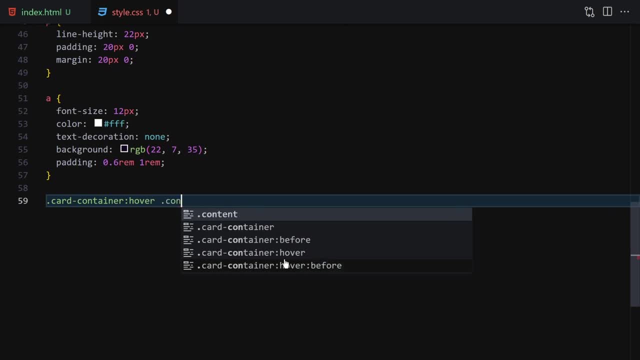 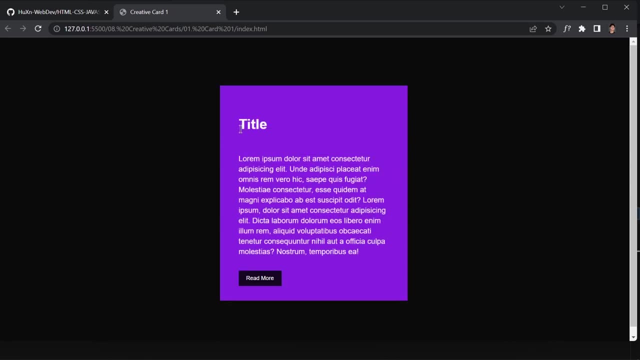 container once you hover over turn. so you want to select the content and you want to change the color to totally pure white? all right, so once i hover my mouse over turn and this is what's going to happen, i guess i should have to provide a little bit spacing in that one. so now let me 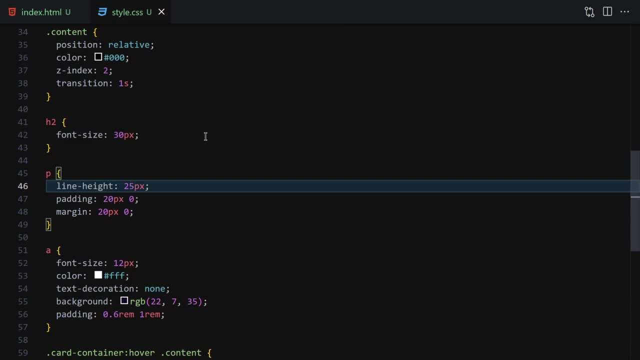 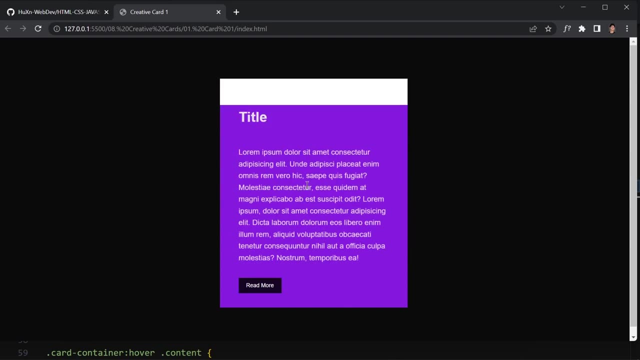 select that. i guess that 25 was correct, but i just changed it to 22, i don't know. all right, so now i guess that's looking cool, much cooler than i was expecting. all right, so now. this was the first project, so now let's jump right into the second card. so now let me review the code a little bit. 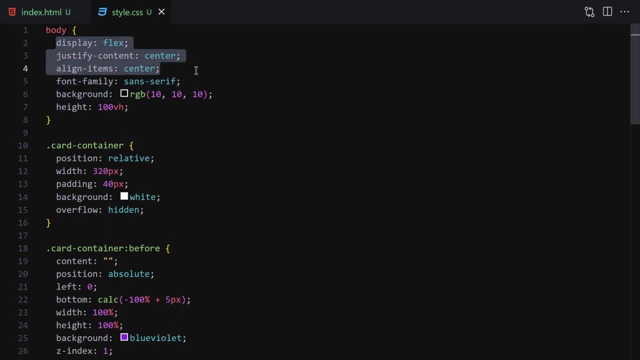 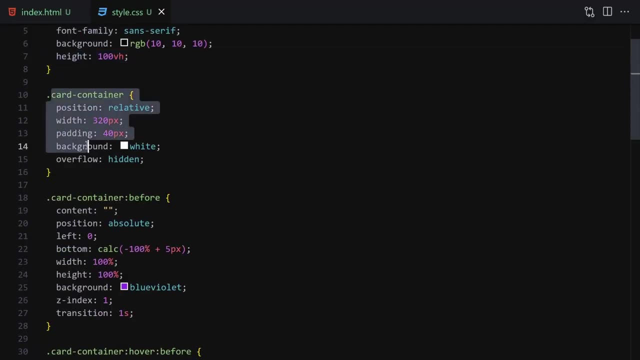 so the first thing we treated: we select a body, we just center everything, we change the font family, we provide a background color, we just provide a height to it, and this is that background stuff, right here. then we select our container and then let me just zoom out a bit. 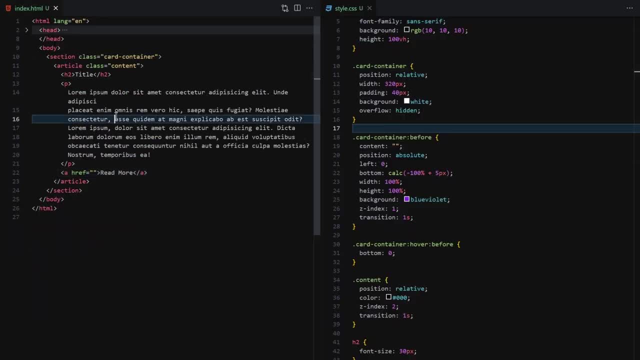 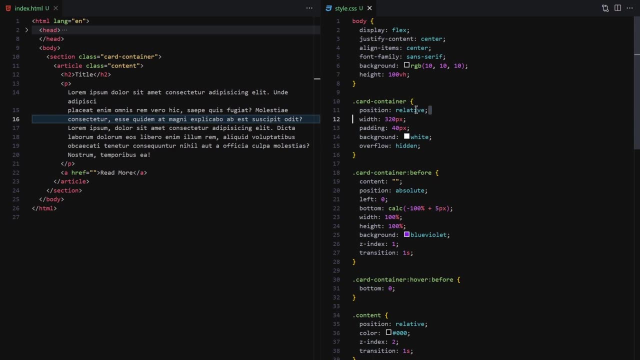 so that you guys can see the html css together. then we have like, uh, okay, that container, this container which i'm talking about. so now the position will be relative, because we want to use before selector and inside this before selector, we are going to be using position absolute. so 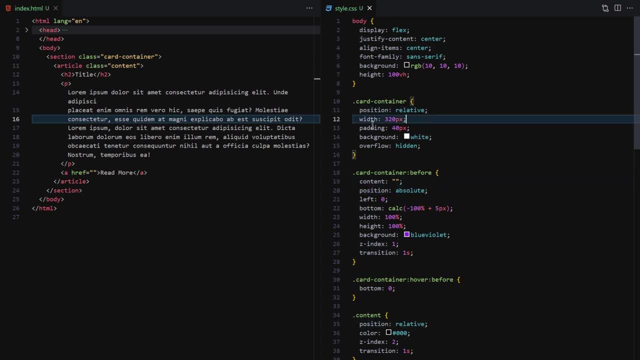 that's why we provide a position relative to it and we also give it a width of 320, so it will just take that much width. and then we provide a padding to it at 40 pixel and we give a background color of totally white. so that's why we are getting a. 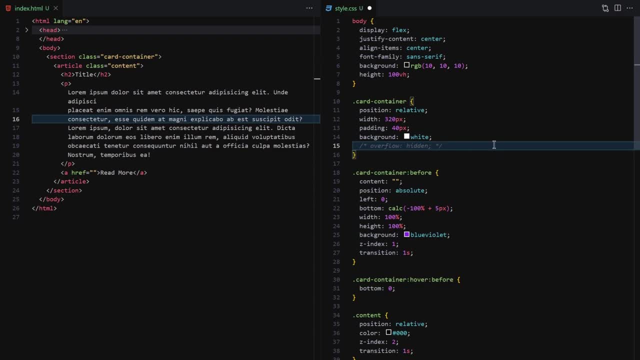 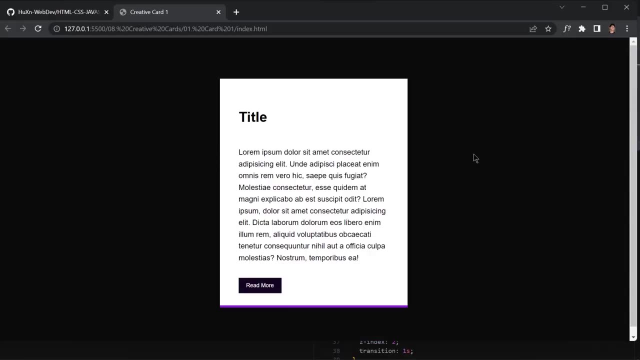 totally white background and if you just uh come in this overflow hidden, save it and this is what's going to happen, all right, so this is what's going to happen. so if you just provide overflow hidden, so this is our card looking like, all right, so then we have like we just uh provide a before. 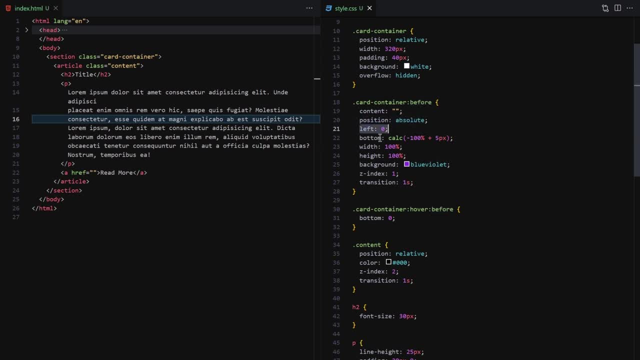 selector trade and then we provide absolute left will be zero. we just use this uh call function right here, and if you guys don't know about call function, i guess i have to make a video on that one, because i didn't explain that call function in my course, html, css course. anyhow, i don't know. 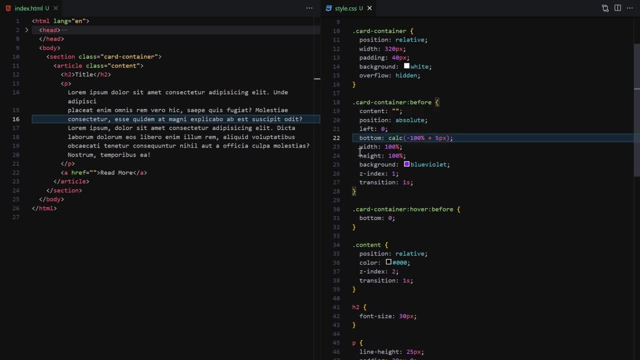 i'm gonna just make a video on that. it's not that much difficult thing. then we have a width and height and it will just take the entire width and height right. here we give a color of this, uh, blue violet color you can give a name of like color of crimson if you want to. so whenever we have a mouse, 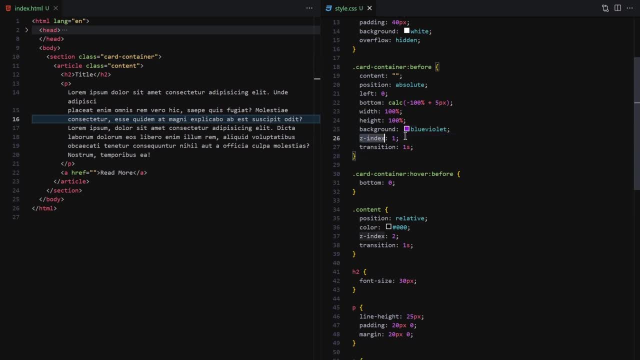 order, so this looking a bit ugly. then we have a z-index uh over here, and then we have a z-index over here, and then we have a z-index over here and then of one right here, and we also just provide a transition of one second because we want this. 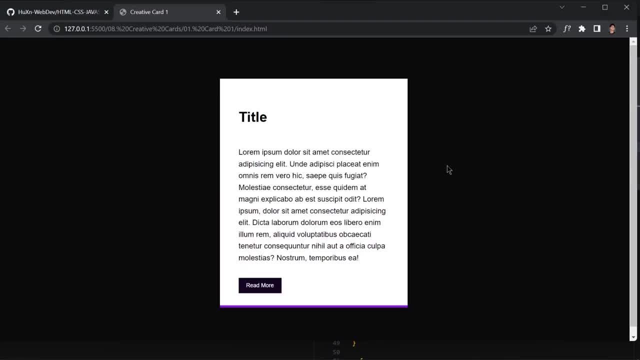 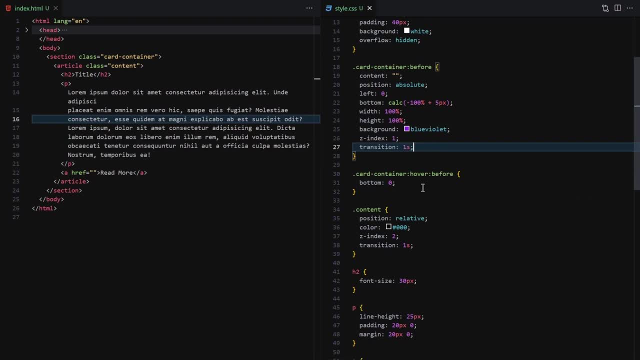 animation to happen smoothly, so like, let's suppose, if i just comment this animation, so here you can see it's going to happen like: uh, it will take more than a half second, so that's kind of ugly. so you want our animation to happen a bit smoothly, so that's why we provide a transition of one. 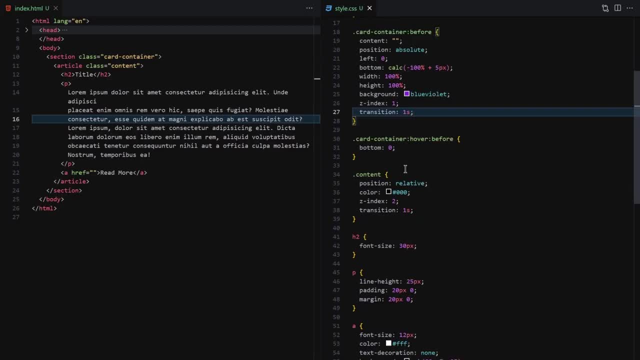 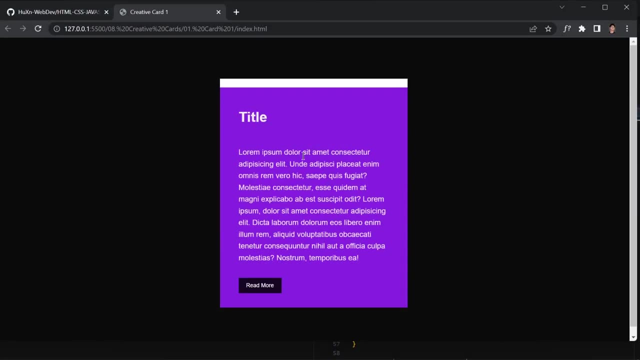 second. so here you can see the transition of one second. all right, so then we have a card container and we have a before selector, so the bottom line will be just taking the zero space. so whenever we hover our mouse over to it, so we'll take the entire space. and then we have a content container. 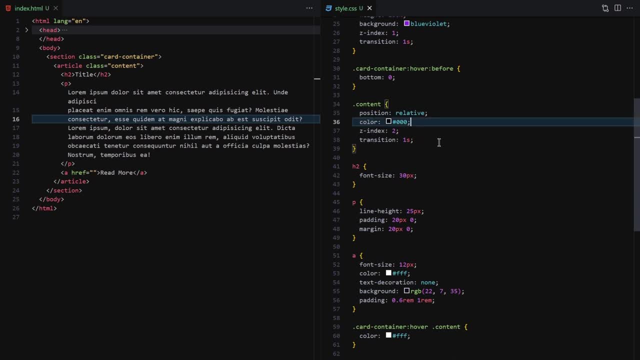 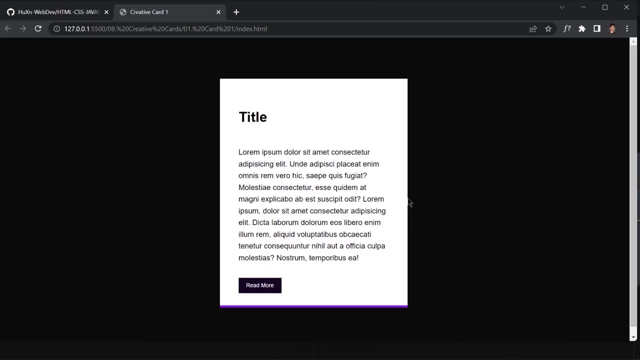 the position will be relative. the color of a black z-index 2, transition 1. and we just formatted our stuff right here and then, once we hover our mouse over to it, so we'll just change the color to white, pure white, right here. okay, so this was the first card, so now let's jump right into the next card. 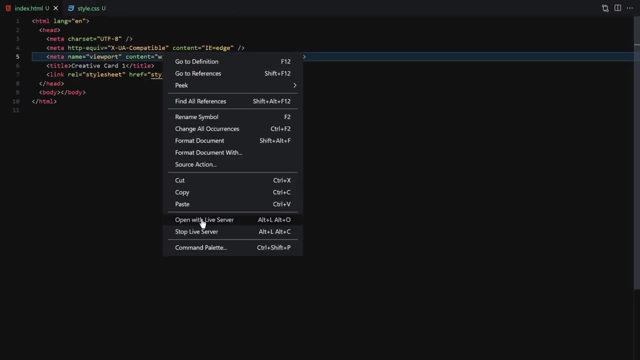 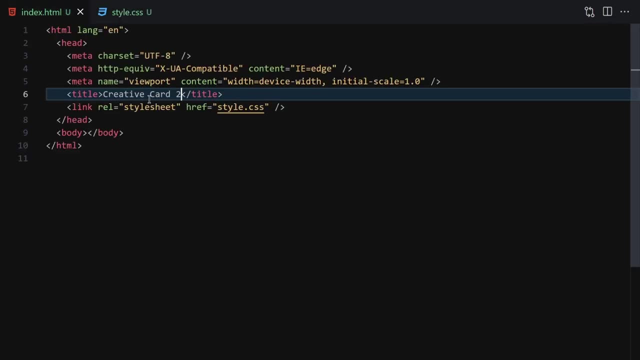 which is this, uh, other one. so now let's just uh open this, and this one will be card two. zoom in a bit so you guys can see everything. and now let's start working on our html. all right, so for html, i will just write a section. 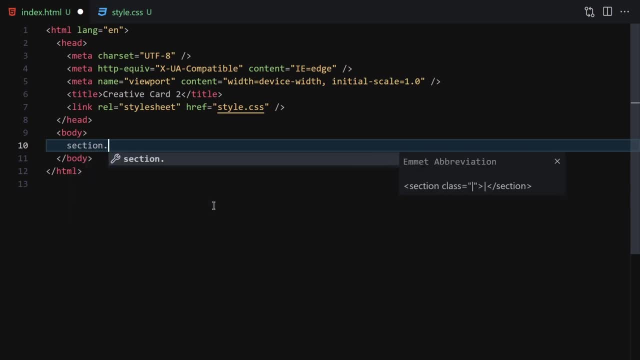 section with the okay section with the class of card. inside this card we are going to be just writing, like a section with the class of image box. okay, inside this image box, we are going to have to have an image. i'm going to just remove that and, by the way, i'm going to place an image. 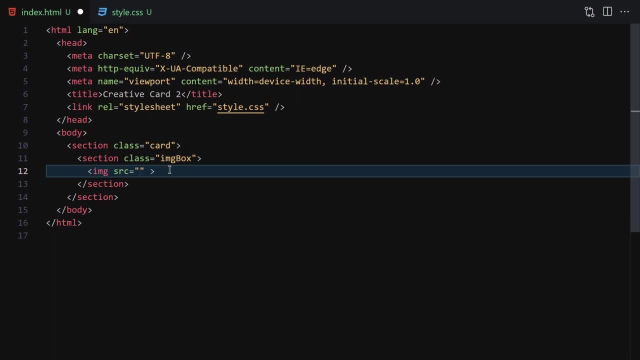 right here and then i'm going to move it from placed to an image folder inside this image folder and we are just going to close our dustbinimage. ok, we now we've done that. e don't we want that. e now we right here, and you will also found this image in the description area, so just click on that. 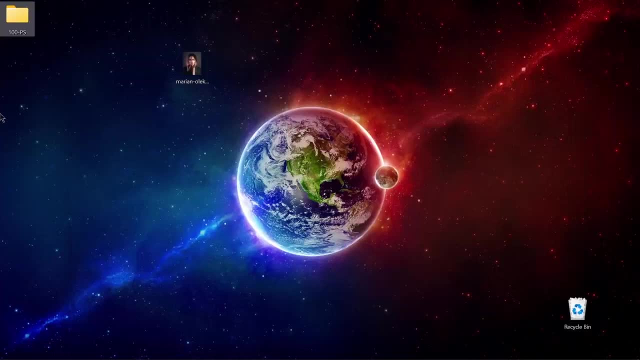 link and it will bring you to my github repository and you can just download this image from there. or you can just go to this link right here and like go to unspash and then just paste this name. it will give you this image right here, or you can just place your own image if you want to. 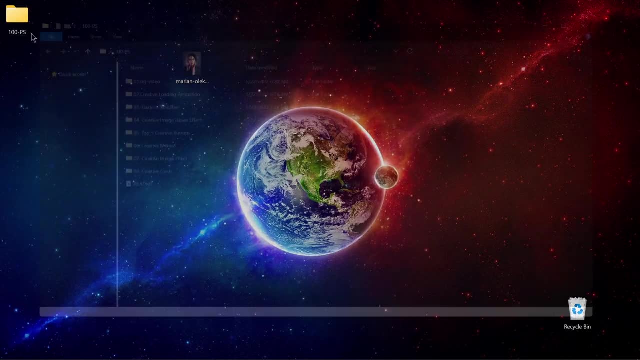 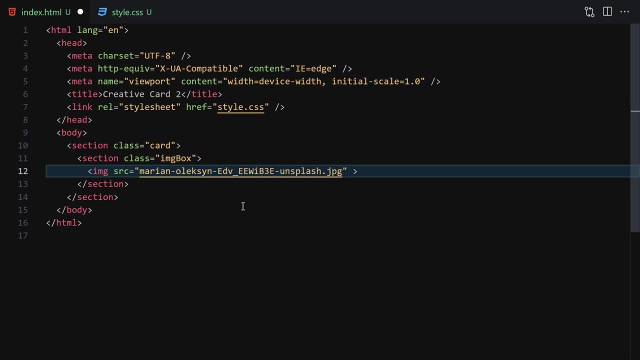 but i have this image, so i'm going to use this one. so i'm going to cut that from there and paste it in the card too, okay, so now i have access to that image right here, so i'm going to place it right here, okay. outside from this section, i'm going to use an article, and with the class of article. 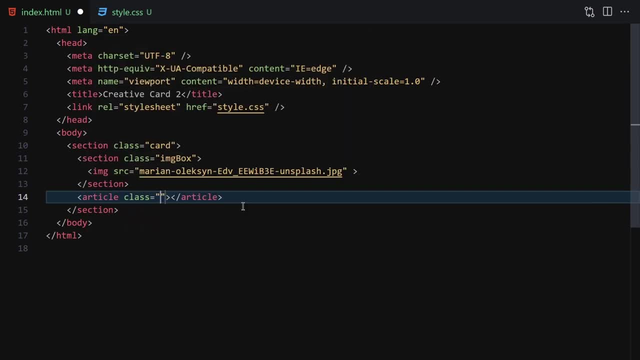 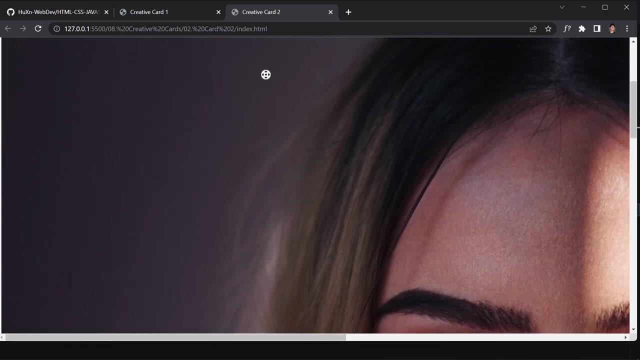 article with the class of details and we would go to h2 of like, uh, i don't know, olivia would be fine, okay, so we have this girl image right here, okay, and then we have her name right here, olivia or whatever her name is. so now let's jump right into it. 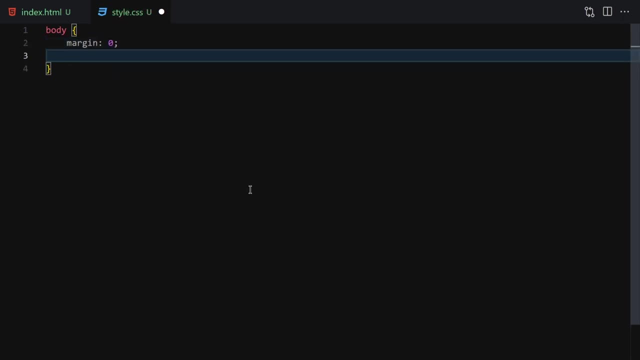 okay, so now let's jump right into it. okay, so first of all, let's select the body. margin will be zero, uh. height will be 100 pixel, 100 vh. background will be linear and gradient- linear linear gradient. and then i'll just pour linear gradient of like. i don't know, i have already set a linear gradient right here, so i'll just use like. 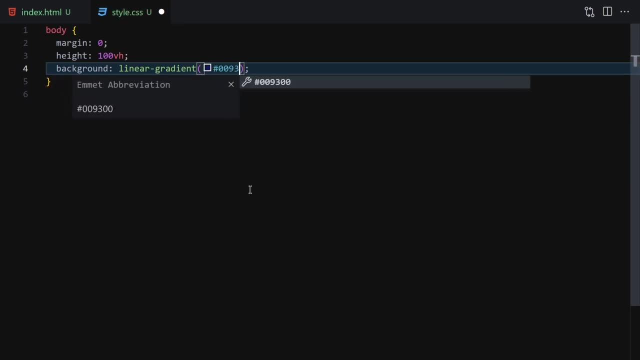 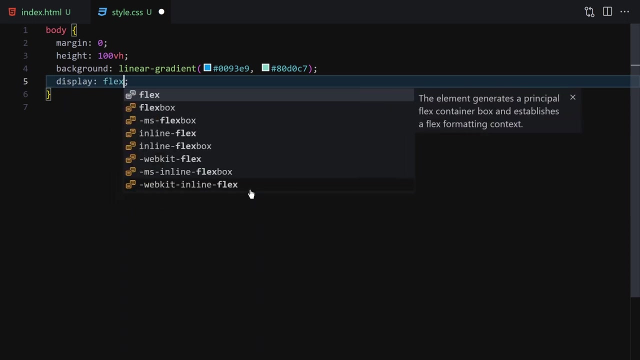 zero, zero, nine, um, three, and then e9, e9, yep. and then we have another gradient which is like: and zero, d, zero, uh, c, seven, okay, so this is the linear gradient. kind of hard, uh. then i'll just for a display of flex. you want everything to be perfectly centered, so that's why we are centering it, and then i'm 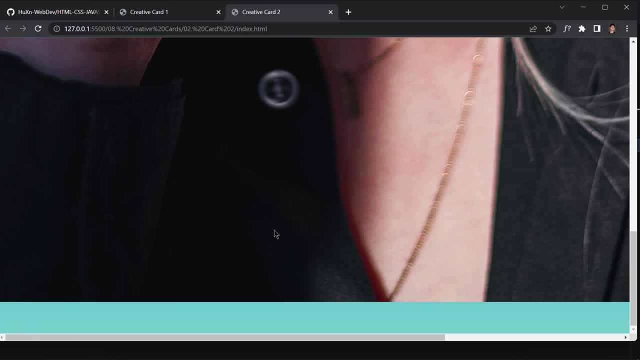 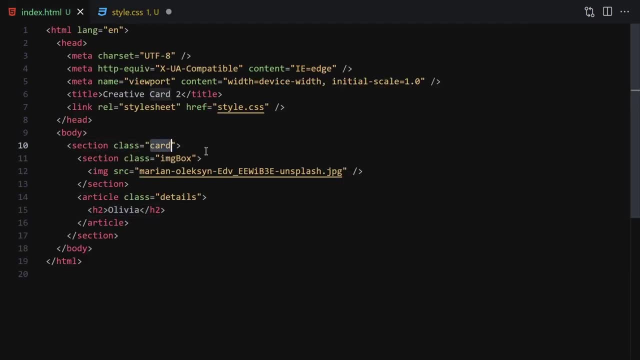 going to choose the form family of sensor and you can choose whichever form family you like. okay, so now we select our background, we change the color, where, and now let's select our card, which is this card. okay, so the position will be relative because you are going to be doing a before and 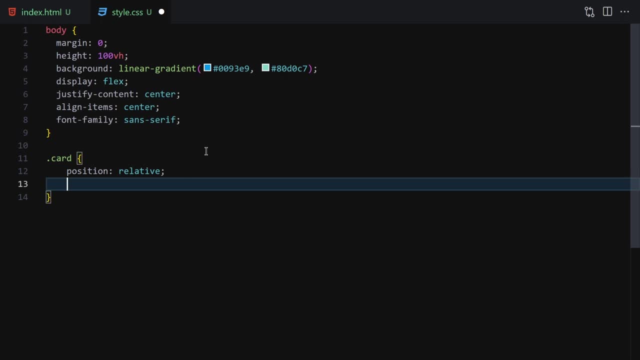 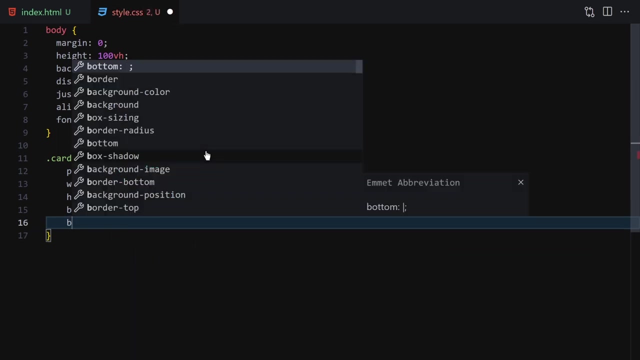 after selector. so that's why you are, we are forwarding the card and then we are going to do a position relative right here. the width will be 30 ram, duplicate it and the height will be also 30 ram, and the background will be white, um, white, white and then the box shadow. 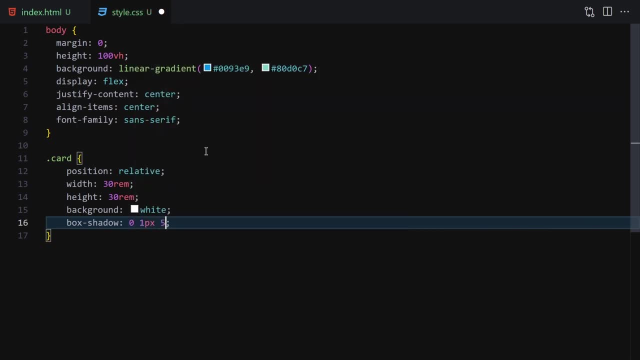 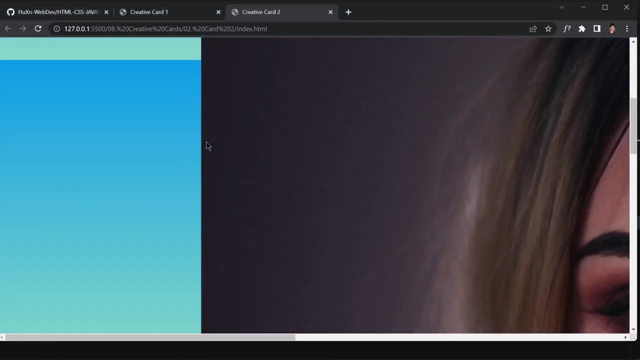 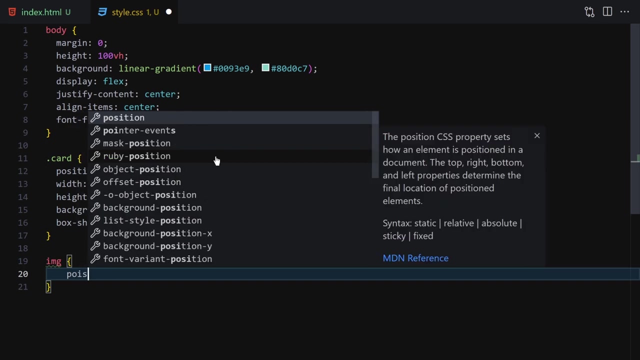 will be just zero, one pixel, five pixel, rgba- zero, zero, zero and 0.5. okay, save it. and we cannot see that because her image is really massive. now let's change the image to, like, a little bit small. so image will be position, position relative, not relative. but 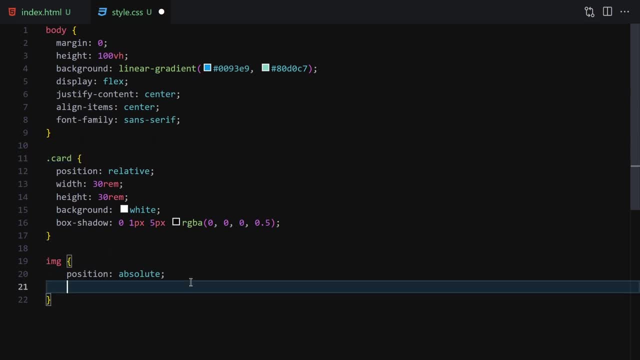 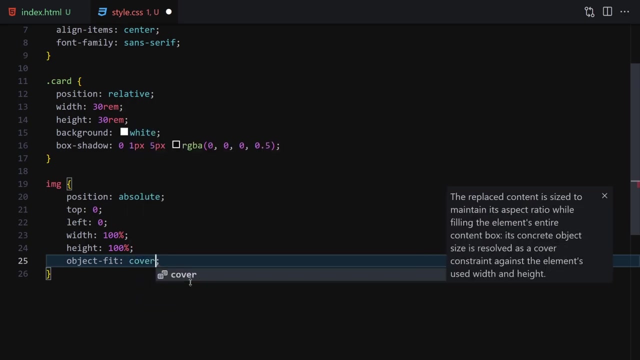 absolute, because you want this image to be inside this card. and now let's make it like: uh, top will be zero, uh, left will be zero, and then width will be hundred percent, and then height will be also hundred percent. and finally thing which you have to do is to just write like object fed. i'll just 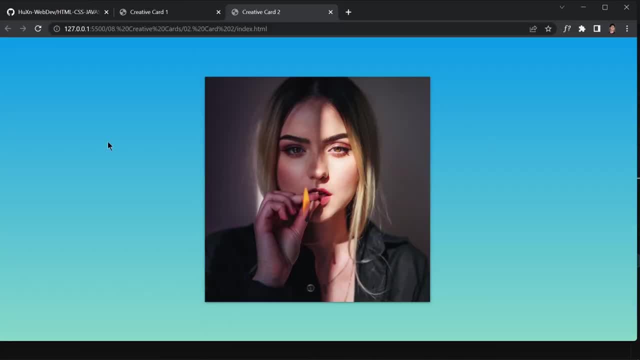 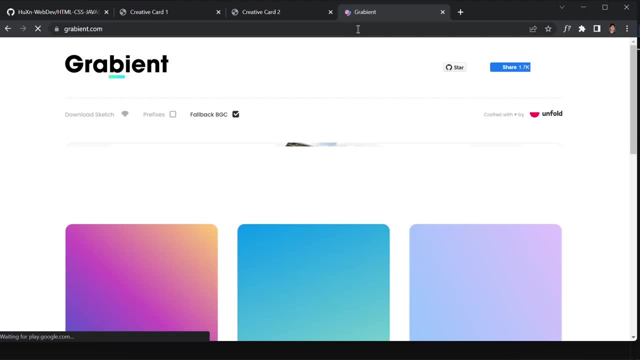 cover it, save it. and now here is our image right here, and here is the linear gradient which we provide right here. okay, you can choose whichever linear gradient you want, and so if you go to this side, it will give you a lot of gradient, cool gradients, so you can just click on that. 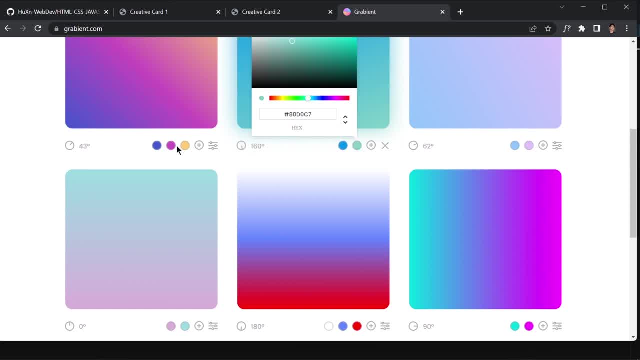 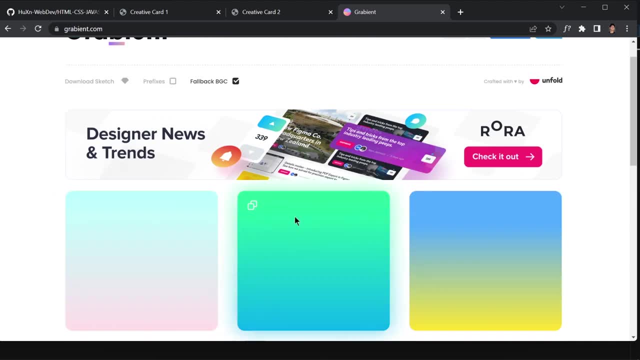 and this is the first color, this is the second color, or you can even go nested colors, like three colors, like one, two and three. you can choose a lot of colors, uh, gradients from here. so here is the gradient, like you can just choose whichever gradient you like. i guess this is an open source. 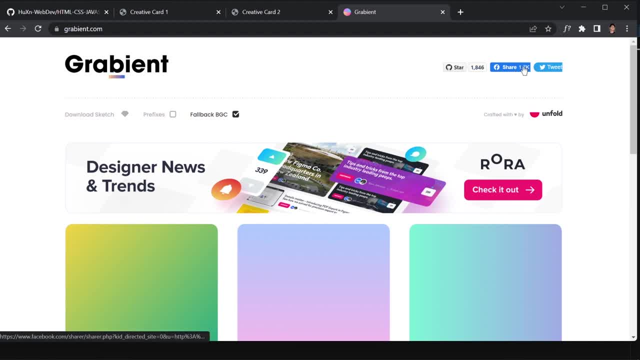 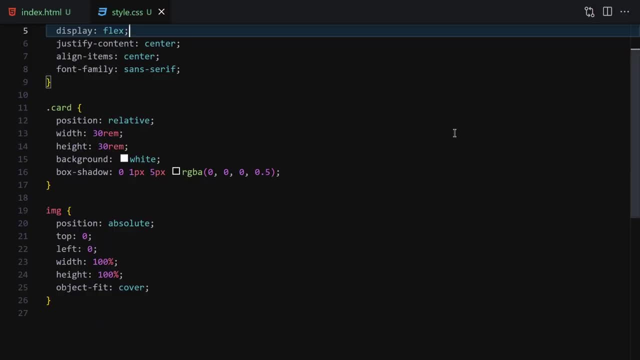 you just have to give a star if you want to. you have a github repository. you can give a star and you can share it by facebook. you can just treat it. you can do whatever you want with it anyhow. so i've choose this gradient from their website. so that's why i'm shouting out to their 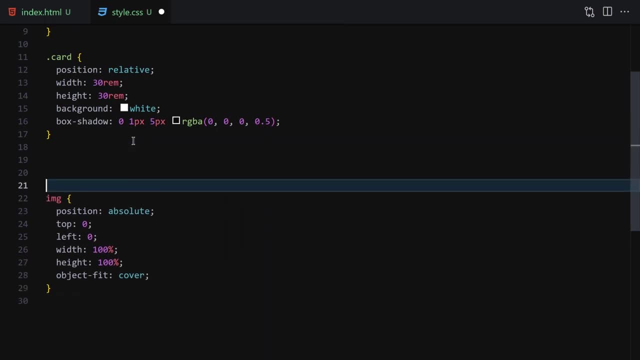 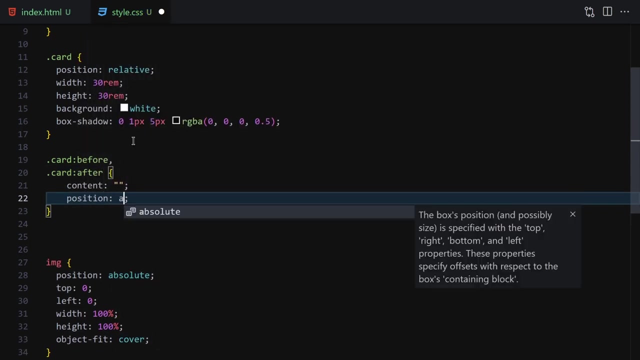 website. so this is the image. so now let's start to do or before and after, selectors. all right, so i'm just do like: card before and then i'm going to duplicate it and card after. remove that column from there. comma and content will be nothing. position will be absolute, so the top will. 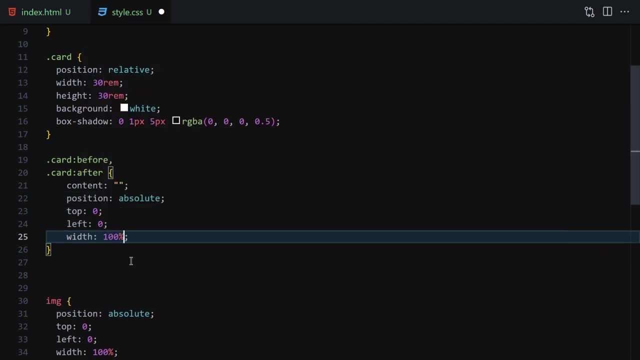 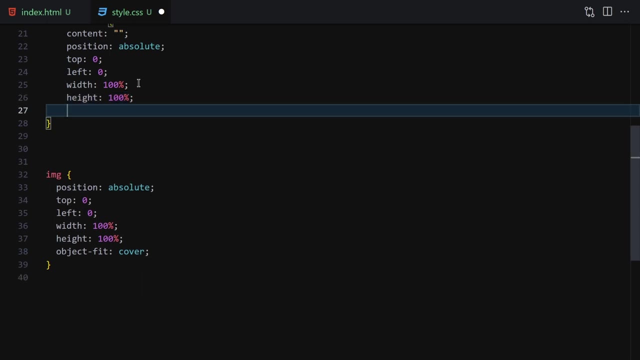 and the left will be zero and the width will be hundred percent and then the height- okay, i just messed up a bit- height will be also 100 and then the background color a bit totally white, and the transition will be just one second and the z index will be minus one. save it and nothing's. 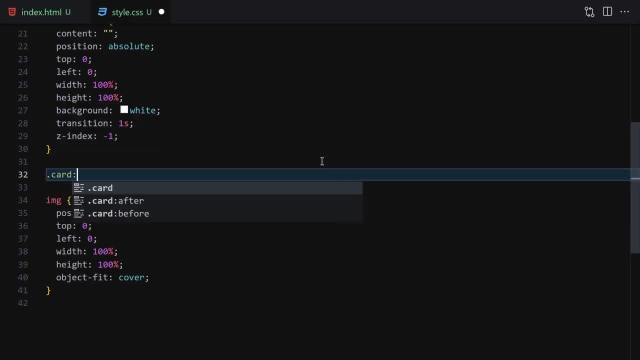 gonna happen because we can provide any hover effector, so i'll just write card hover if we hover over to the before selector. so you just provide a transform of root rotation: 20 degree. we'll just provide a rotation of 20 degree and box shadow: 0, 2 pixel and 20 pixel and rgb: a zero, zero, zero, zero point two. save it. and now let's check it. 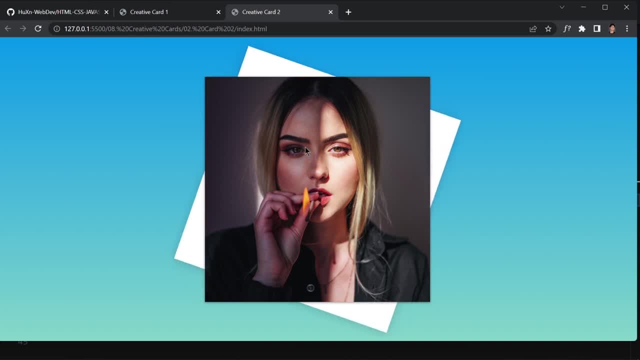 so here you can see, here we have the first card, and now we also want to do with after effects, not adobe after effects, but the after effects. so now here, if you hover over to it, we get a single card right here, but we want to duplicate it, so i'm just duplicate. 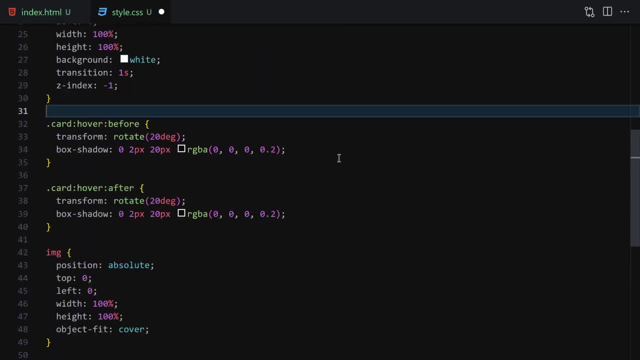 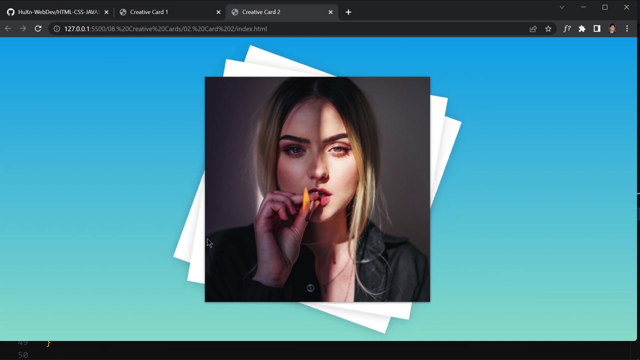 it and change this one to like after and the rotation will be 10 degree instead of 20. and yeah, i guess the box shadow is fine. save it. and now, if you hover mouse altered. so now we we are getting two uh cards beside this girl right here. okay. 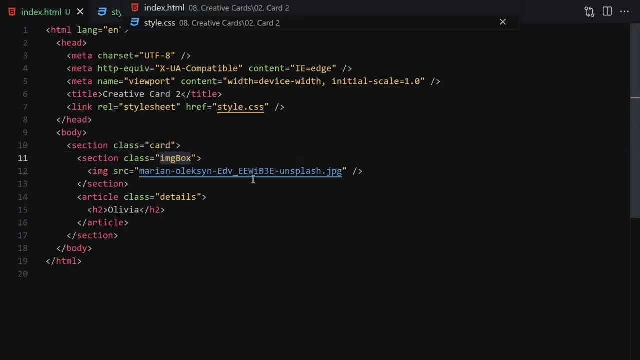 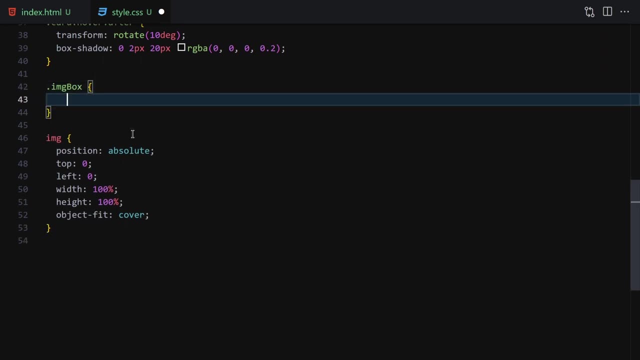 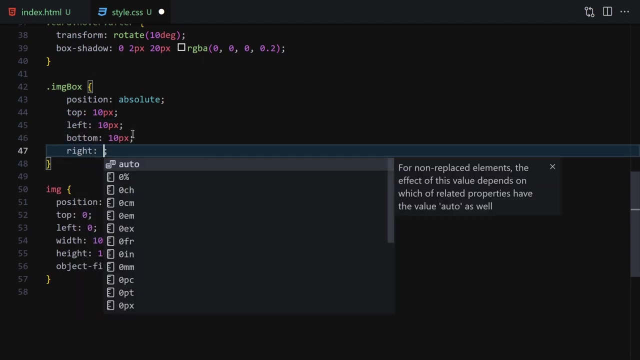 so now let's format this image box right now. so go to there and now let's select or start image box, and now we have to just provide a position, position of absolute, and then top will be 10 pixel, uh, left will be 10 pixel and bottom will be 10 pixel and right will be also 10 pixel. 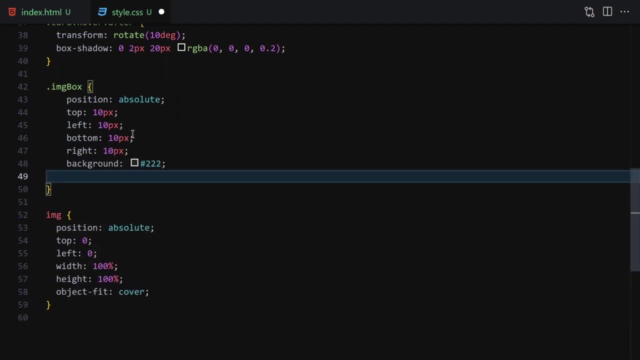 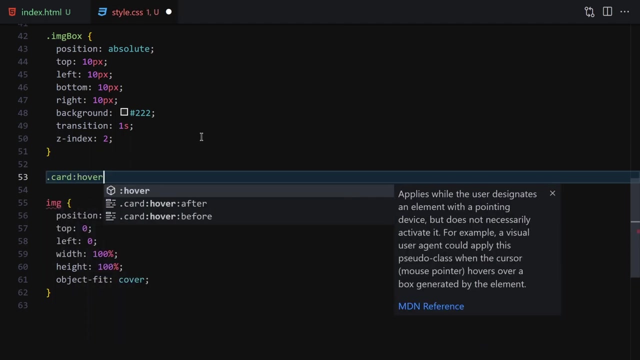 background color will be just this. two to two and then transition, because you want to provide a hover effector. so we have a one second transition. zero index will be two and save it. and now you want to also just provide a hover effector, so like i'll just use like car once you hover over the image box. so 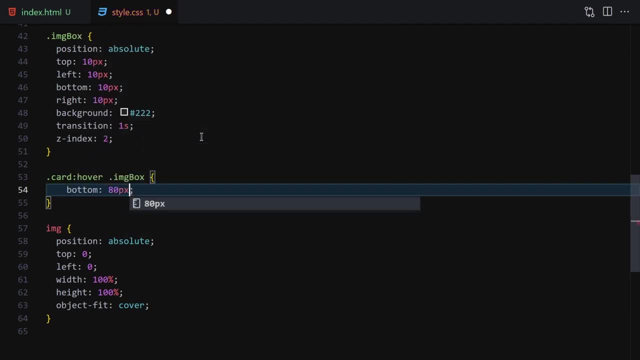 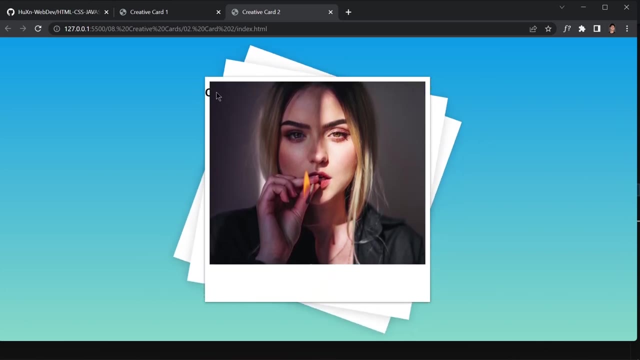 you want to just get the bottom to like 80 pixels, save it. and now, once we have our mouse altered, so here you can see, it will gives us the effect. but here you can also see the text which we wrote inside here: her name. so now let's just center this details container. so now let's. 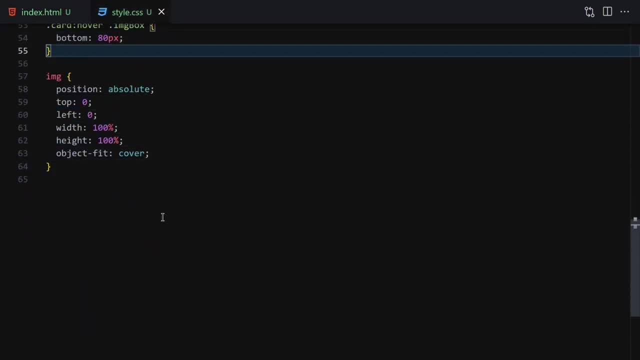 format this digital container. so i'm gonna have to go a little bit down, so i'll just use like d tails. was that correct? yep, details, details, both of them are fine. position of this one will be also absolute, and left will be 10 pixel, right will be 10 pixel, bottom will be 10 pixel and. 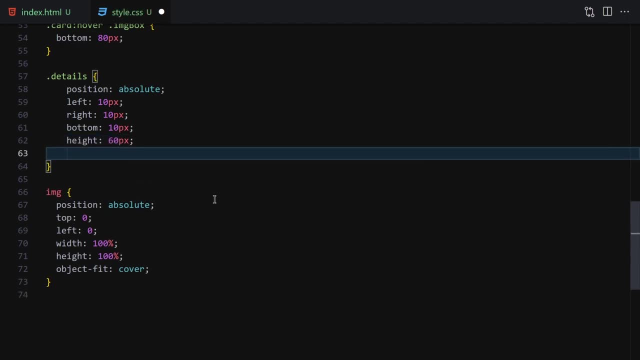 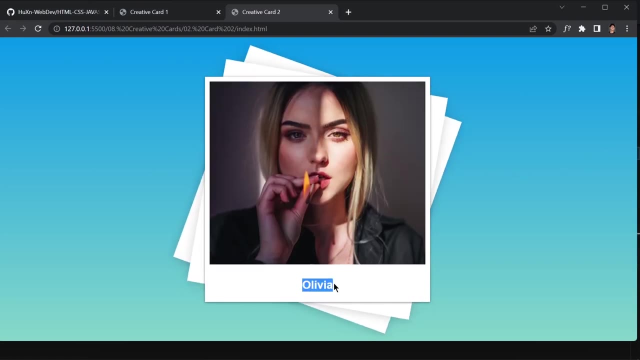 height we will give is like 60, maybe 60 pixel, and text align will be also center. save it and now, once you have our order. so here you can see, we are now getting her name and these three cards right here. so this is before, the other one is after and this is our actual card and this is. 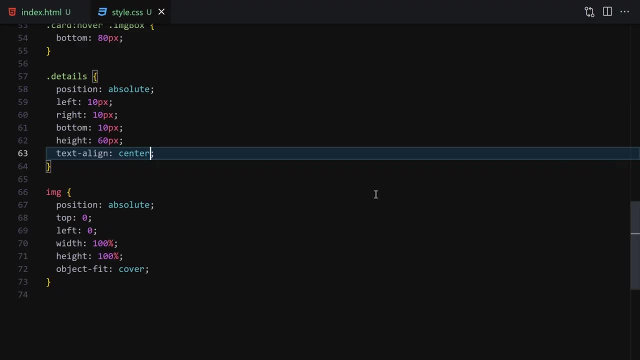 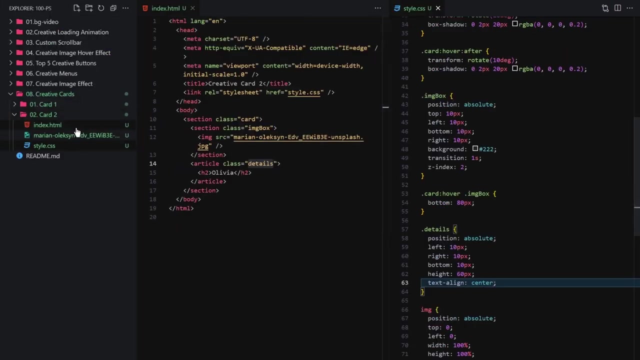 her name, which is center. by the way, there was a lot of talking. i don't want to talk, no more. i mean, like my throat is sweating, all right. so that was the first project, so now let me just review all of the code one more time, and then we are going to be good to go. so, by the way, you want to use your. 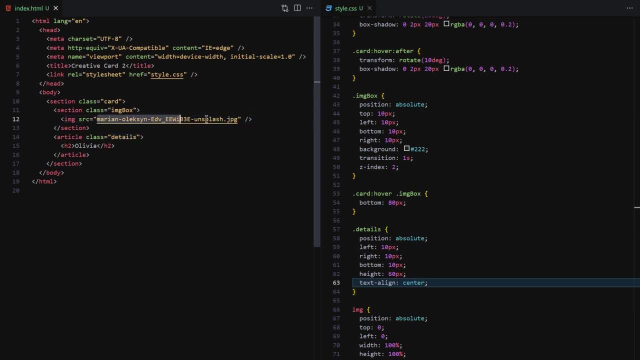 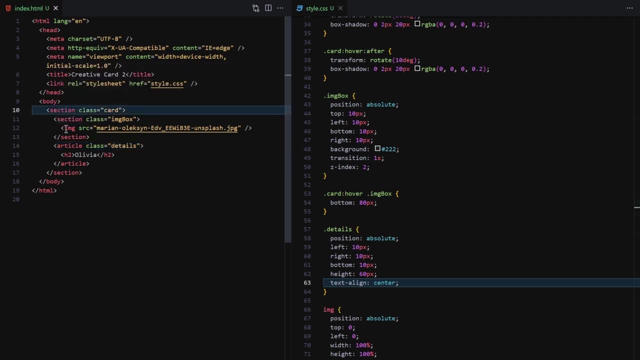 own image so you can also use your own image. i just uh take this image from unsplashcom shoutout to as well. so the first thing we have is a card container. then inside a card content, we have a section with a class of image box. then we have an image inside it. then we have an article of 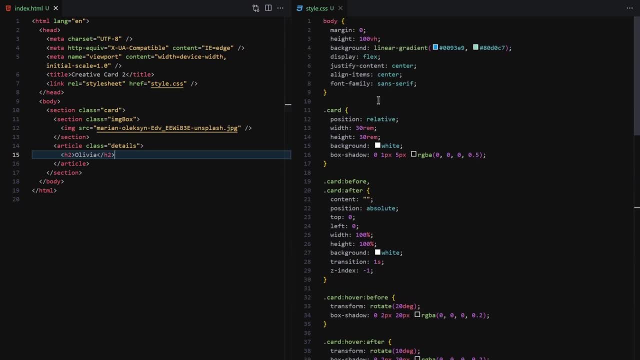 with a class of detail and then her name. okay, so the first thing we treated is we just provided a linear gradient to it and we just centered everything and we changed the font family to sans serif and we give 100 vh heart. okay, then we select our card, we put a position relative to it. 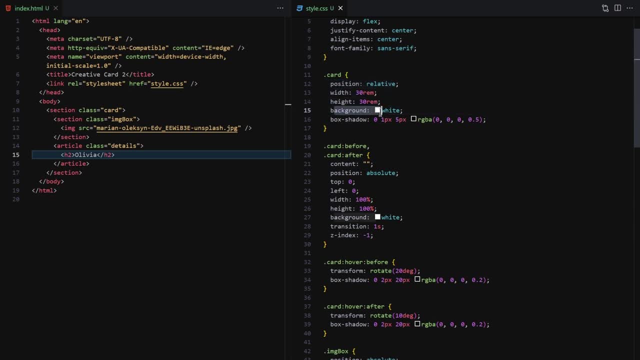 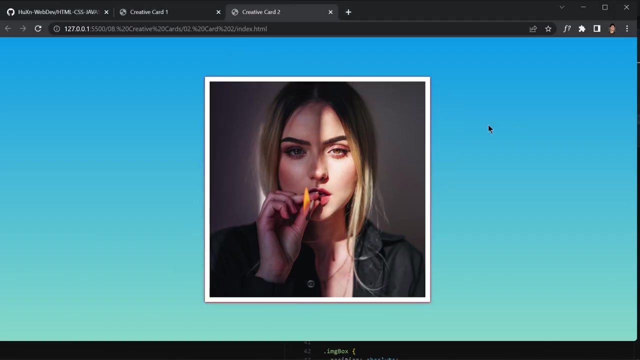 we give a width and height of 30 grams, we give background color of white and then we also put a background, the box shadow. this is the box shadow. let me just show you that, like i don't know, blue will be fine and you cannot see that blue. let me just change this to like red, save it and now here. 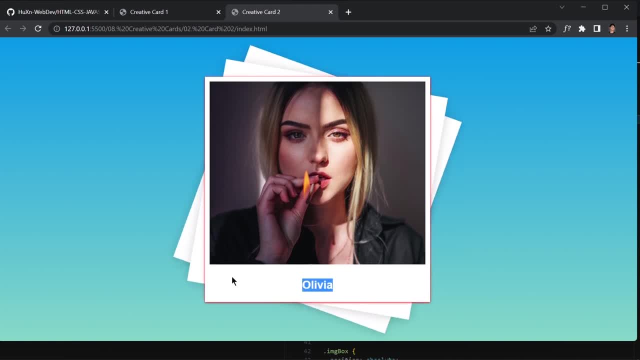 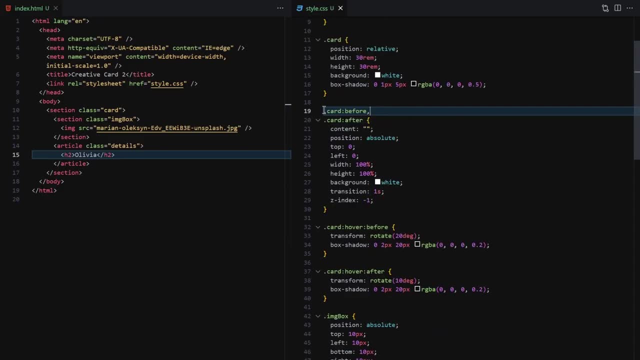 you can see that box shadow is just like light box right here. so if i just undo it one more time, so this is our box shadow here. you can see that. all right, then we use a before and after selector. we provide a position. absolute to top left will be zero and width and height will be the same. 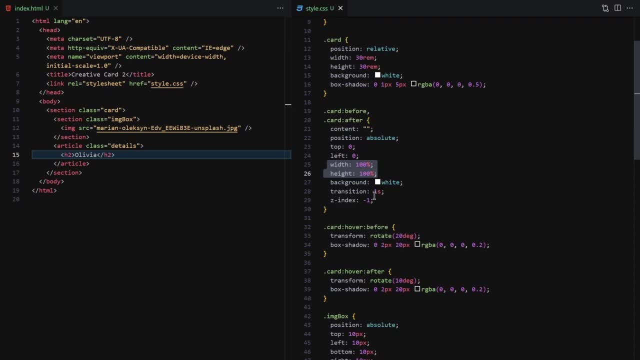 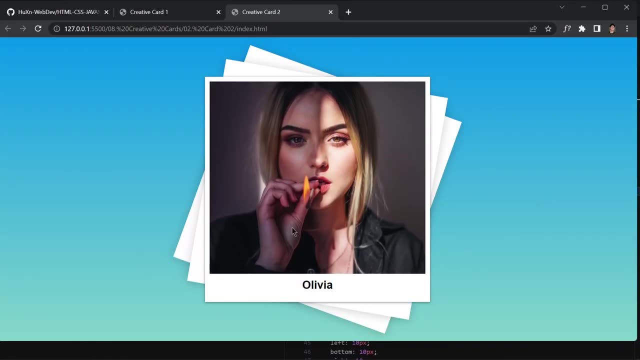 as this card, and then we have a background color of wire. transition will be one second because you want the transition to happen smoothly, save it and then it's really going to happen like this and this is not looking cool. it's looking more than ugly. so you want this to happen a bit smoothly. 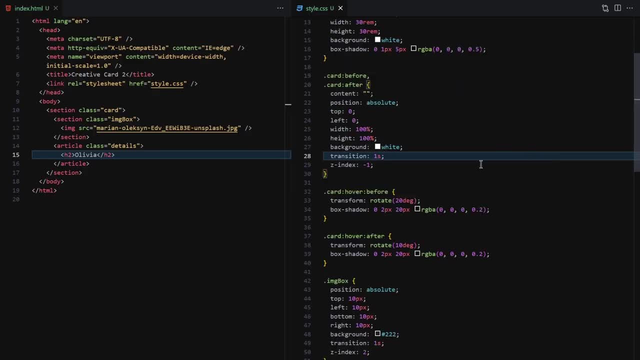 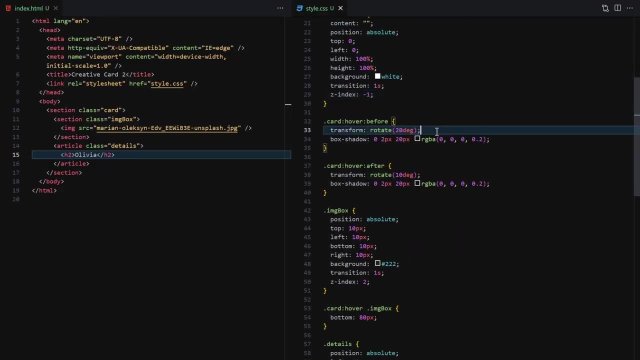 so that's why we provide a transition of one, second, third. then we have a z index and which will just show everything at the top. then we have a card hot effect. we just rotate this first card to 20 degree and we rotate that after a car to 20 degree and we rotate that after a car to 20 degree. 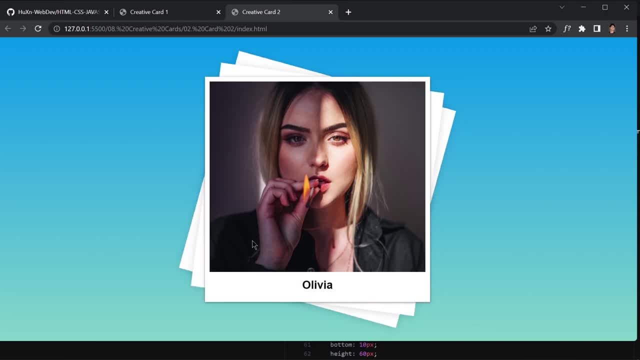 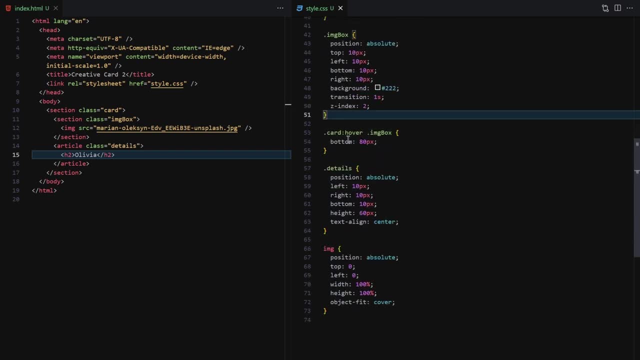 10 degrees. so that's why we are getting this uh first and second card right here. then we have an image box right here. we provide a position absolute to it and we just format it a bit and then we just provide a hover effect to it. so whenever we hover over to it, so it gives there. 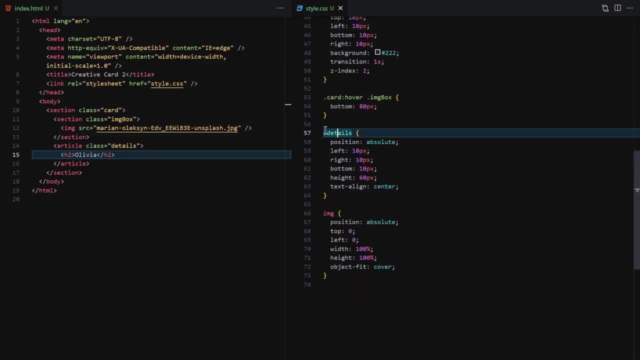 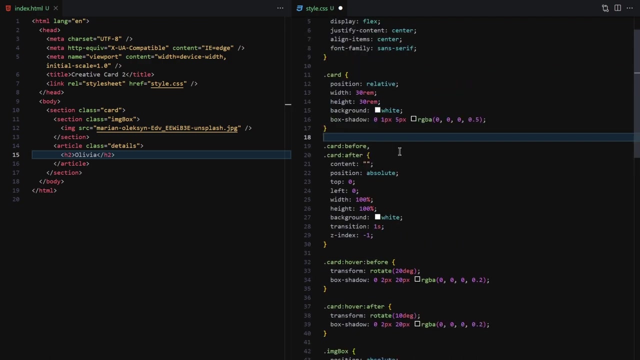 much space and it will take this image. okay, then we have this details container. it allows us to just center our name right here and then we have an image. we should have to take this image from there and paste it somewhere right here. so once we format our card, um, i guess i should have to just put it right here. both of them will work, i don't. 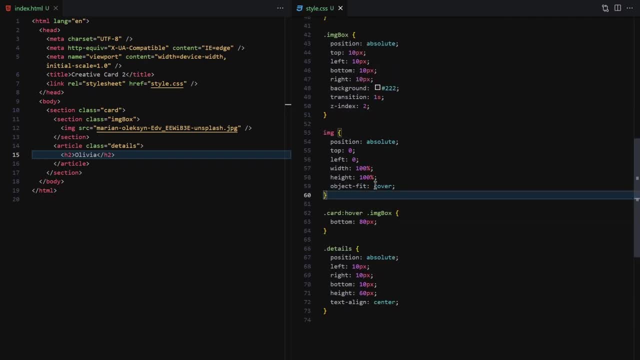 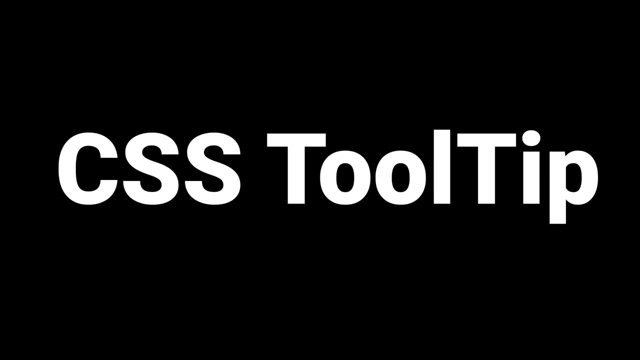 mean like it will not work. both of them will work, but this is just a good style to do it anyhow. so you get the idea all right. so that was the second cards. hey guys, hussein, and welcome to the ninth project of this course. so in this video, 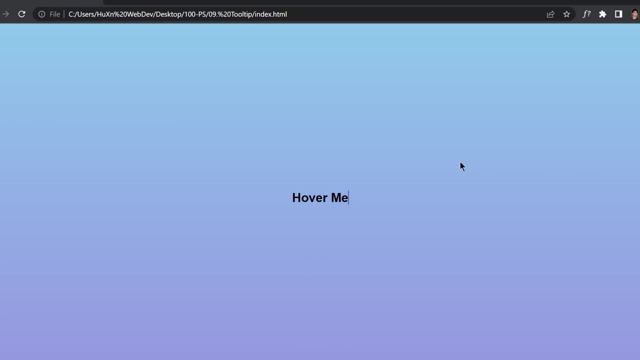 we are going to be just creating this simple tooltip by just using html and css- no javascript, no, nothing. so if you hold your mouse over to it, so we will just create this simple tooltip by just using html and css- no javascript, no, nothing. so if you hold your mouse over to it, so we will just 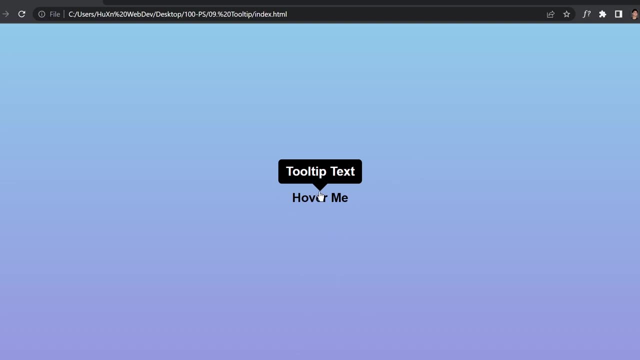 get this tooltip text right here, and if you want to place your own text, so you can also place them, but in my case i just write like tooltip text right here. so this is going to be the easy project of this course. so, without wasting any time, so now let's jumble right into it. and now. 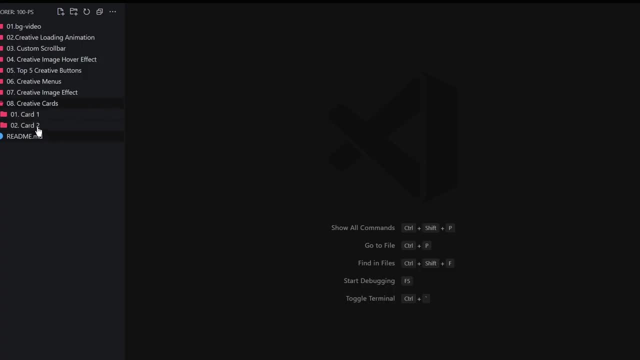 let's just create this tooltip. in the previous review, we've created this- creative cards- but in this video, we are going to be creating a tooltip by just using html and css. no javascript, no preprocessor like sas, no whatsoever, just pure html and css. okay, so what are we going to be doing? 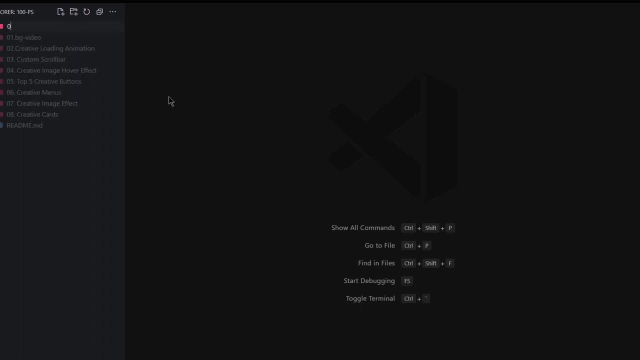 in this video we are going to be creating an archive to create a currentlySixty pdf project just by using an html and css, no javascript, no preprocessor like sass, okay, so what we? so what i'm going to do? i'm going to create a new folder given name of 09 and then tool tip: okay, and 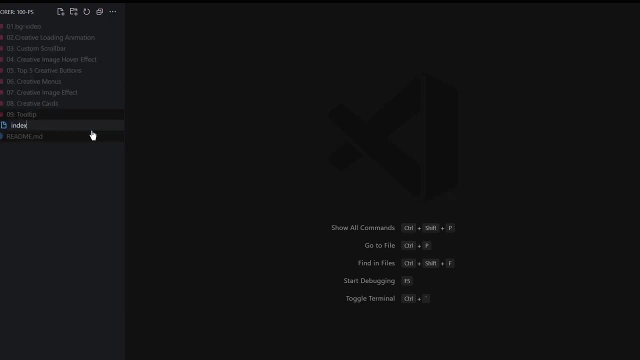 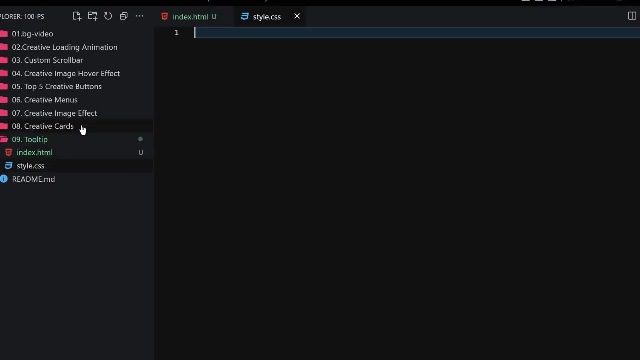 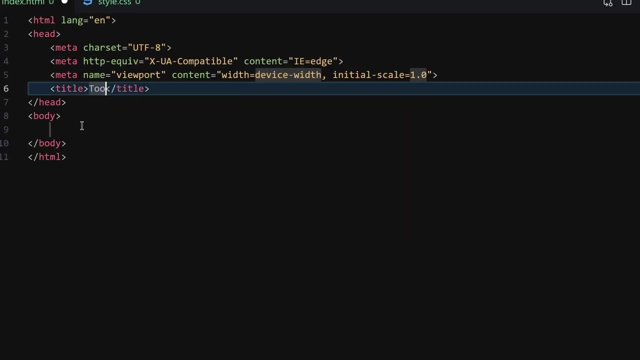 then, inside this tool tip, i'm going to create two files like indexhtml, and then another one will be stylecss. so let me make it a bit bigger so that we can see it a bit better. okay, so the first thing i'll do is i'll just create a doc type and give a name of like tool tip, and then i'll link it. 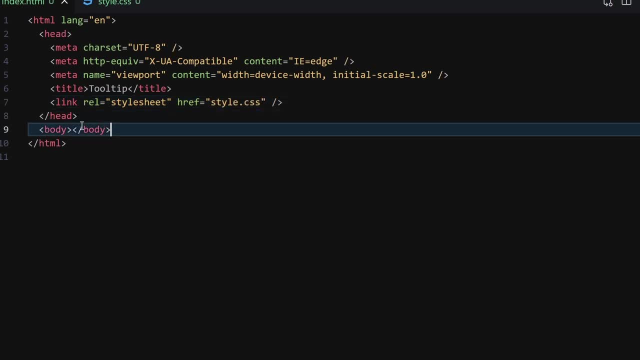 with my css file, save it. and now let's launch it with live server. so i'm going to right click and click on the live server. the first thing i'll do i'll just provide a div with the id of container. okay, just container. inside this container we will have, like spans, two spans. so the first one will be: 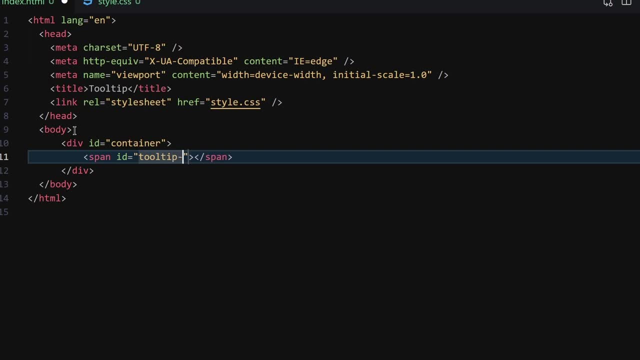 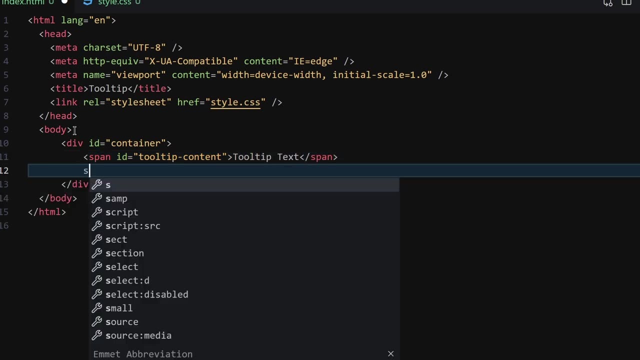 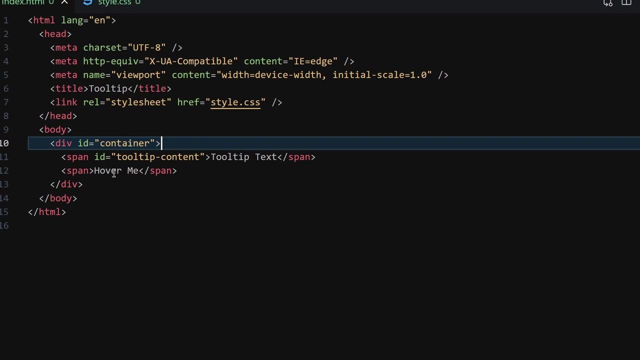 uh id of like tool tip and also tool tip content content. i'll just write like tool tip text and then we will have another span. so i'll just write: span howard me, okay. so this is just a html for this tooltip. so the first thing we have is a div with the class of uh, with the id of container. 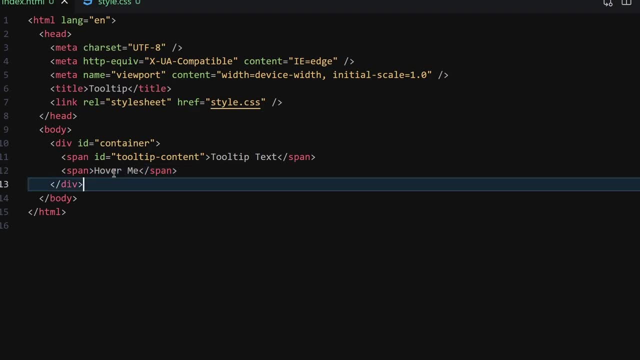 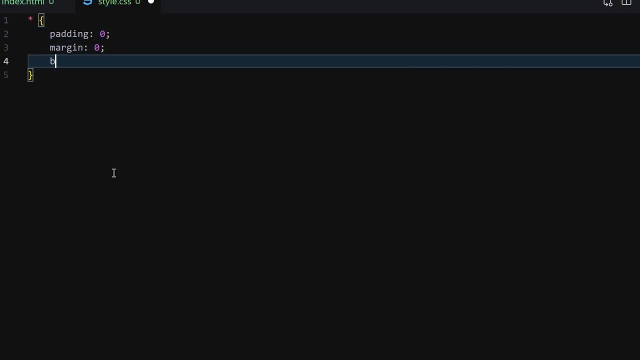 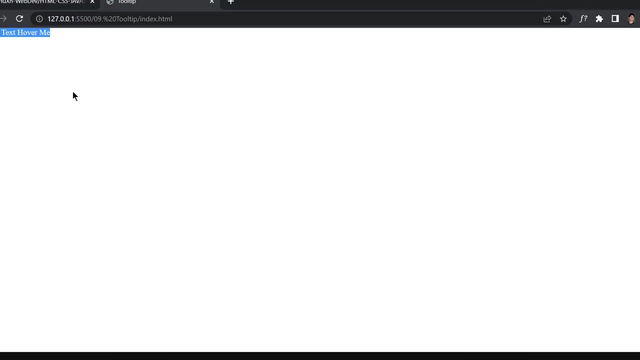 and then we have an id of tooltip content and then we have, like howard me, okay. so now let's jump right into a css, and the first thing i'll do i'll just remove that padding and that margin, just a bit of a reset. and then box setting or box sizing of border box, save it. and here is our tooltip text. 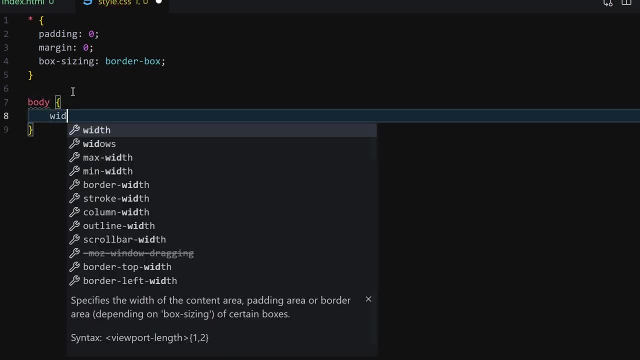 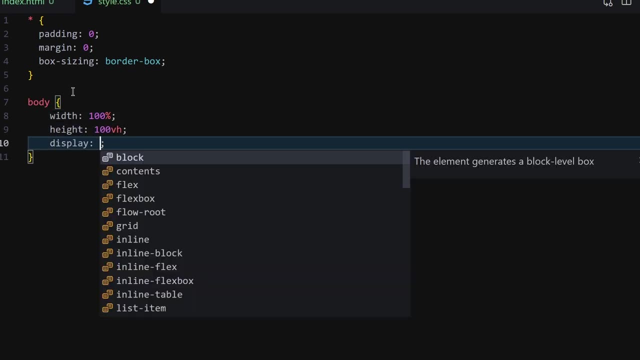 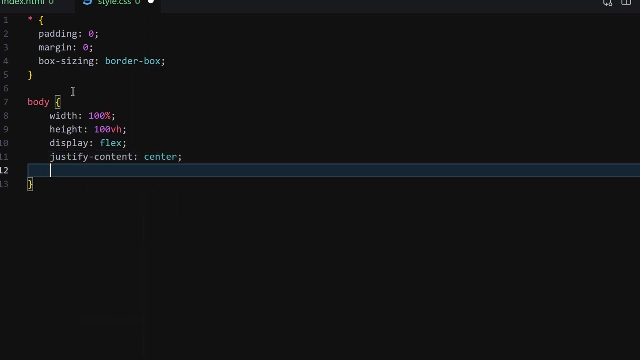 okay, so now i'm going to jump right into the body and i'm going to give him a width of like 100, and then i'm going to also provide a height of 100. vh display will be center, because we want everything to be center. uh, display flex and justify corner will be center. line items will be. 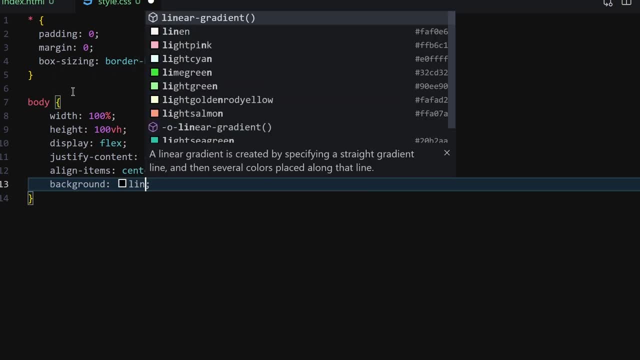 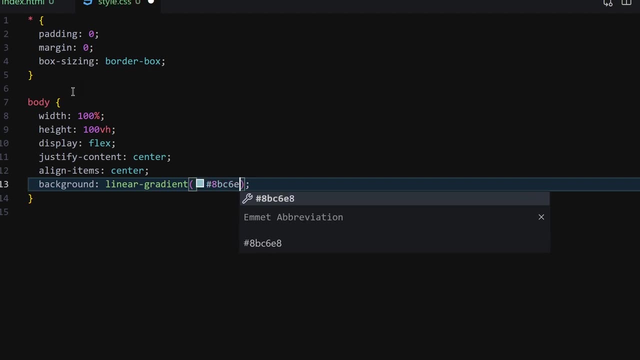 also center and background color will be a linear gradient. so i'll just write a linear gradient and the first one will be uh- adbc, um 6 ec and the second one is also linear gradient. so i'll just write linear gradient and the first one will be uh- adbc, um 6 ec and the second one will be uh- adbc, um 6 ec. 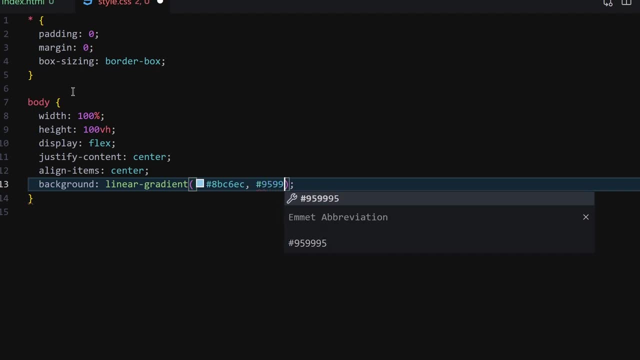 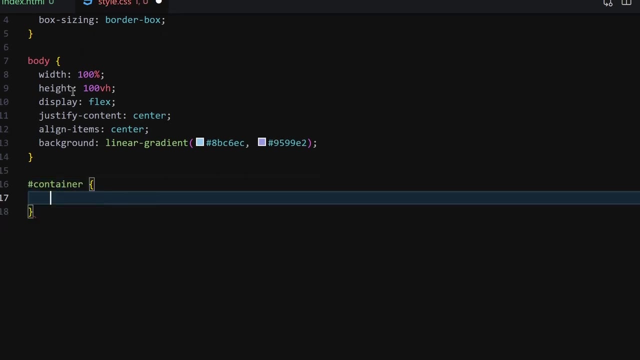 then comma 9599 e2: okay, so this is the color, and now let's generate to the container. so i'll just select that container, which is this container right here, okay, and then i'm going to give a position of relative to it, and then the cursor will be pointer and inside the padding will be: 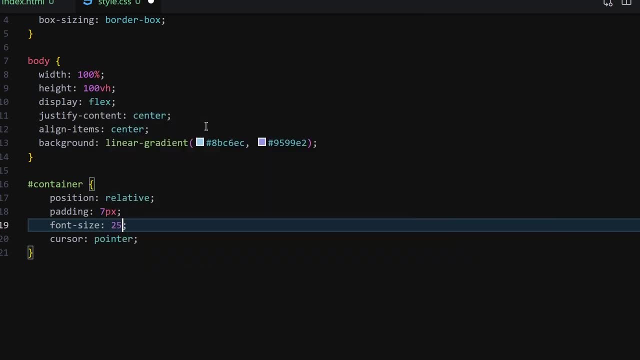 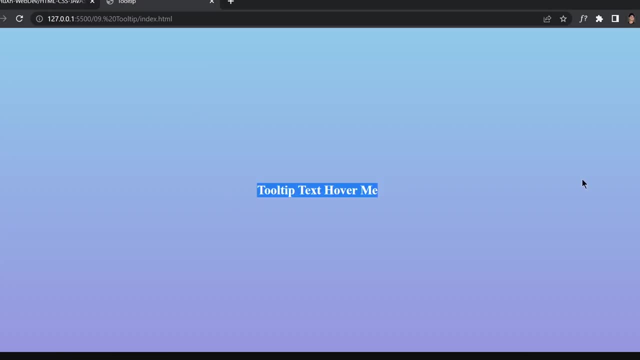 seven uh pixel and then font size. i'm going to make it just a bit bigger so that we can see it. so 25 pixel and font width will be bold. so once we save our file and this is our tooltip right here, okay, and it's now saying like: hover me and whenever we hover over to it, and so our cursor. 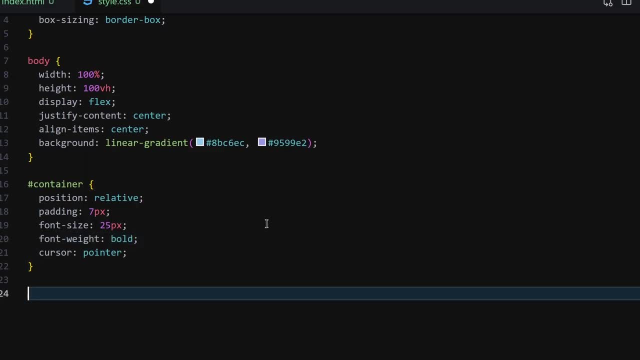 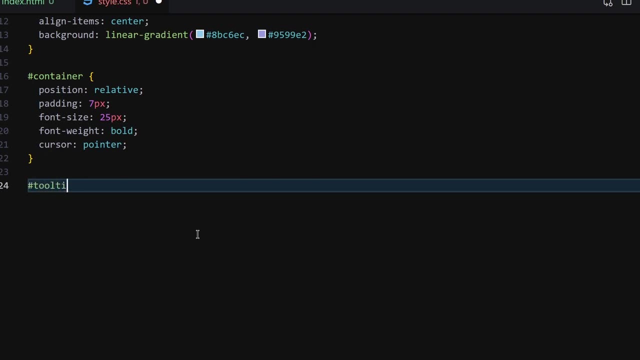 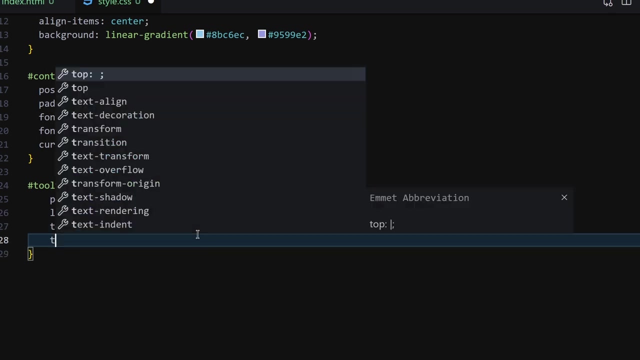 changes to like pointer right here. okay, anyhow. so now let's select this tooltip content right now. so now i'm going to just write like tool tip and then, uh, content, not container, but just content inside there. i'm going to write a position of absolute and then outside the left, 50 percent, and then top will be zero and transform. 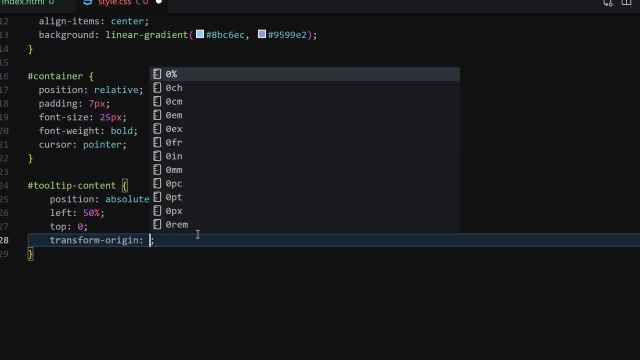 uh, not transform origin transform, just a simple transform will be translate x axis and we want them to be to go like minus 50 percent, and then we have a background of totally black and then we have a color of pure white and then we have a white space. 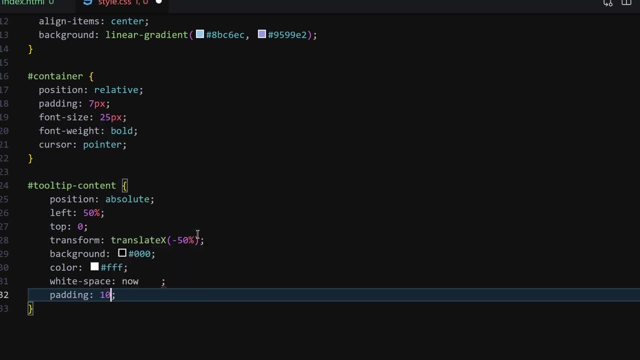 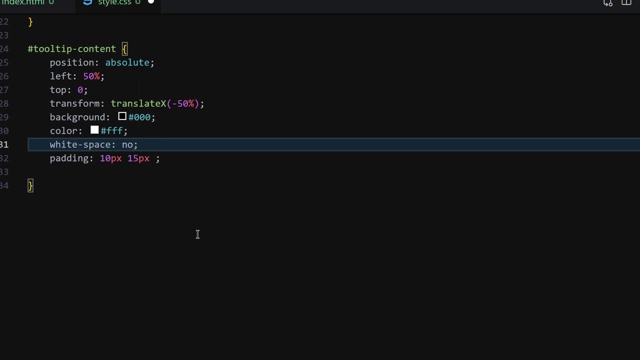 of no right, right. and then we have a padding: top and bottom will be 10 pixel and left, right will be 15 pixel. uh, it should be no wrap, okay. and then we have a border radius of 7 pixel, just a little bit of border. and then we have a visibility hidden currently, it will be now hidden and we have 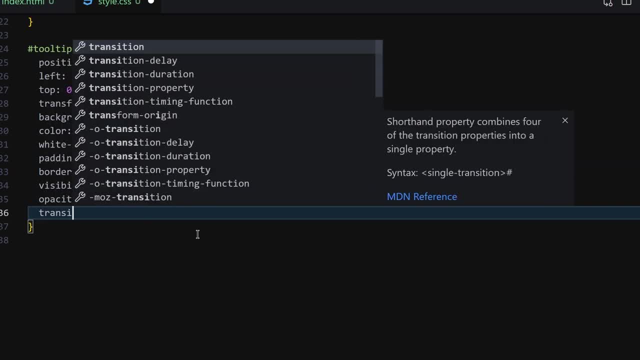 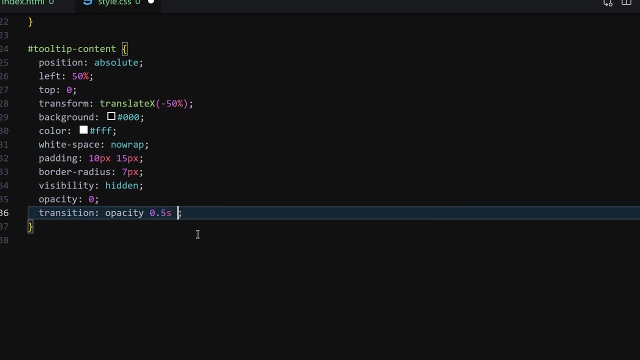 opacity of zero, so it will be totally hidden, and then we also want to provide a transition to it. so transition to opacity, opacity, opacity and 0.5 seconds ease. okay, so that's because we are going to be working with a before selector and we are going to be also hovering over to a content, so that's why we are using this uh transition with. 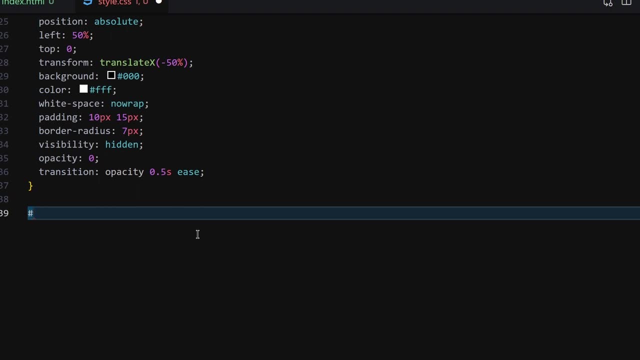 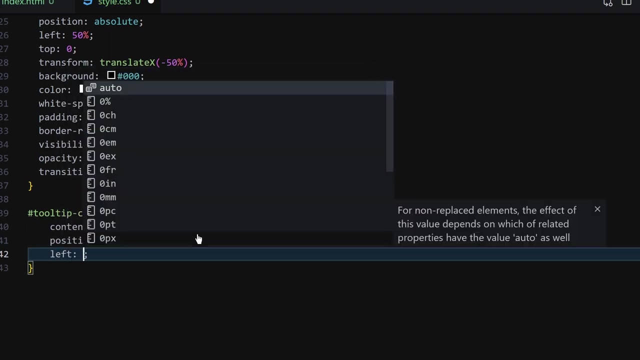 opacity of like 0.5 seconds, because we want our transition to go a bit smoother. so, tool tip content: now we are using a before and then we have to provide a content of nothing, and then we have position of absolute and then the left side will be. 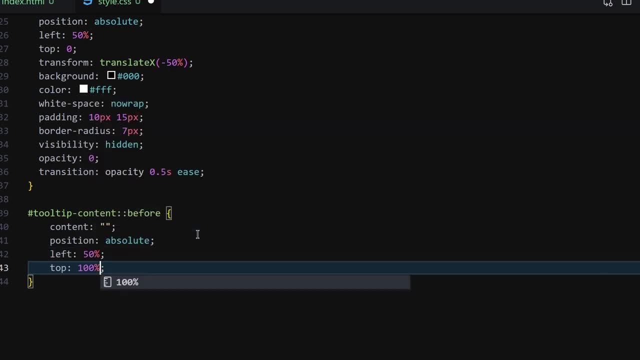 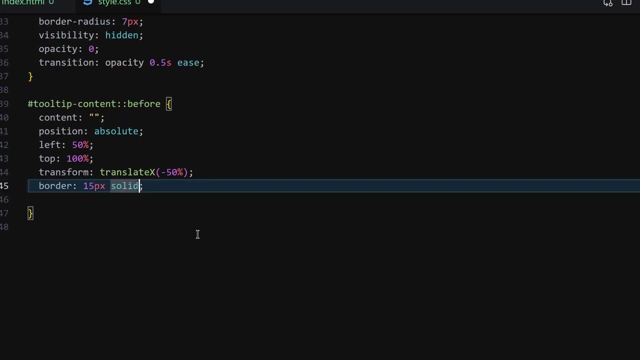 percent and then the top will be, and then we have a transform of translate x axis and then we have a and 50 though filter, 15 pixels Isolated. so you just go with a 15 pixel solid. notice: change the border color two or like a ض� 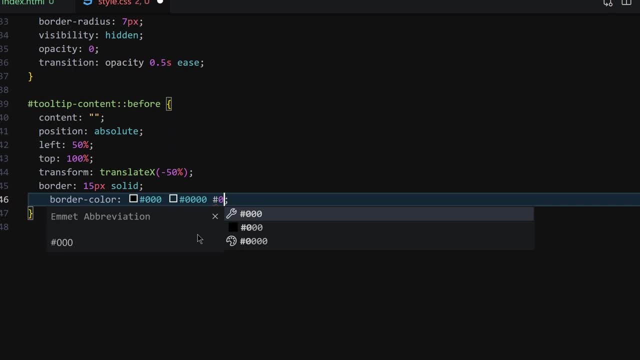 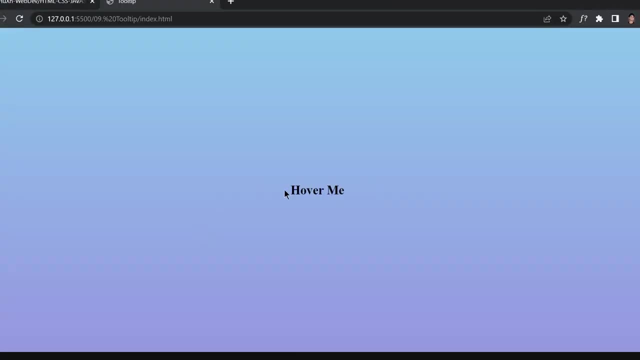 We will see this again. b4 X Obligatory 按 to: And now I changing to one, two, three, four one more time More than supported Pacific set to to Angle TLN of two, three, four this last time. okay, so nothing is going to happen because our tooltip is gone. 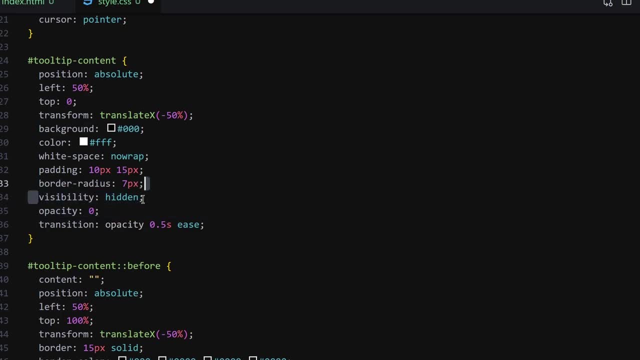 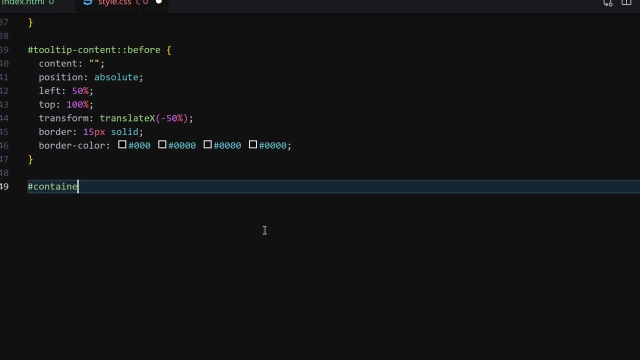 that's because of this um opacity and visibility hidden. so whenever we hover over through this text, so it will just give us our tooltip. okay, so now let's select our container and once we hover over to this container and we want to select this tooltip of content, and then top will be minus. 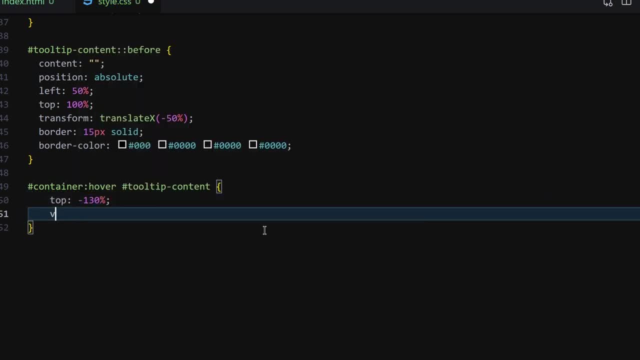 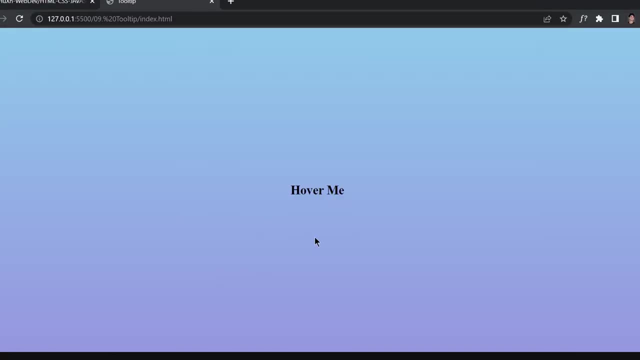 one thirty percent, and then we have our visibility will be now visible instead of hidden, and then we have opacity will be one. so once we set our file, and now if i hover over to it, so here you can see, it will now gives us this tooltip right here, and if you want to change the font, 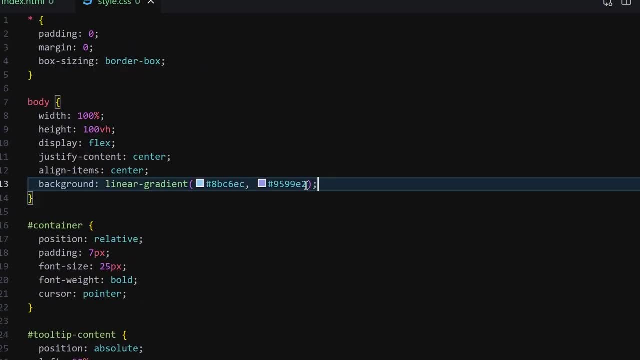 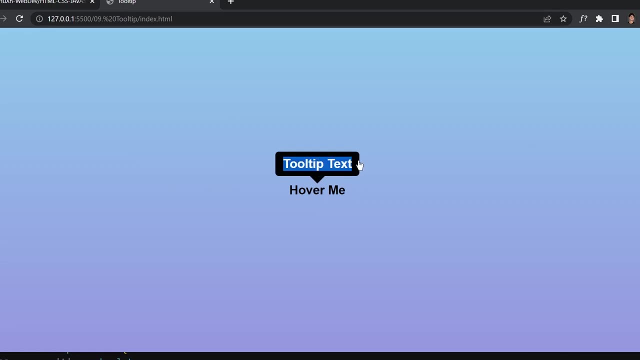 family of that, so you can also change the font family of that one as well. so maybe i should just provide a font family right here. send serif: you can choose whichever font you like, so when i hover my mouse over to it. so here you can see, we've got a simple tooltip right here. and, by the way, if 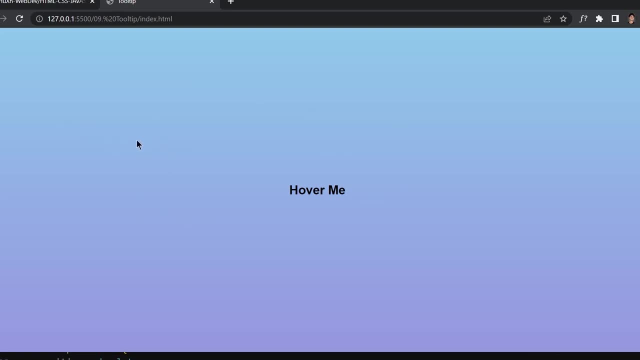 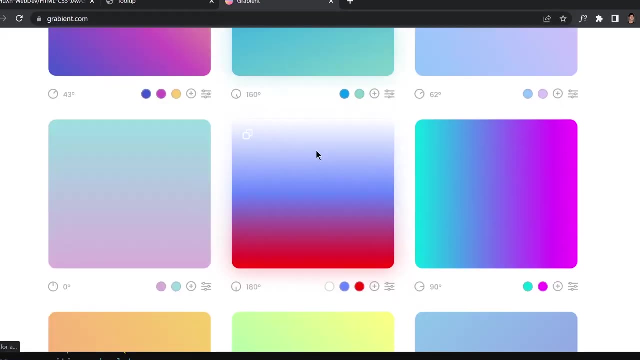 you are wondering, like where i get this um background color. so i get there from this side, which is like if i go to this gradientcom, so here you will find lots of gradient. so here you can see, i guess i choose like jonas guy, i guess i choose this one. i'm not exactly sure, but you can. 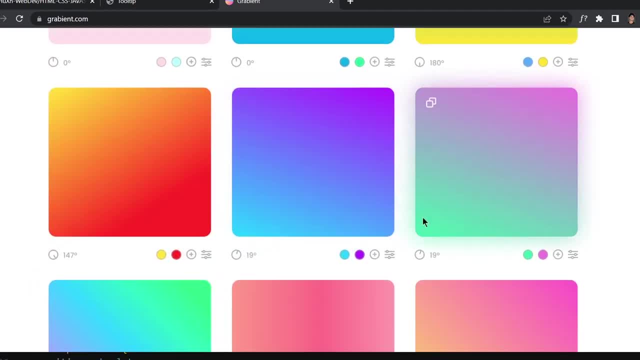 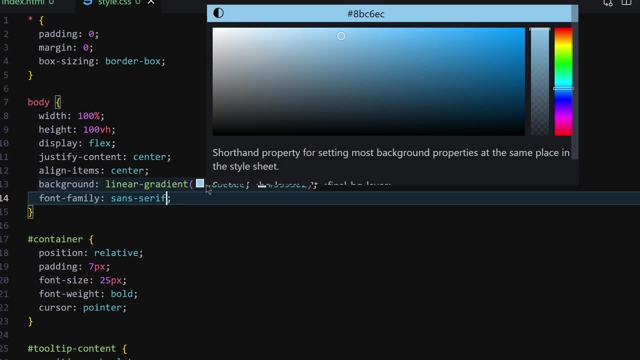 choose whichever you like from there. okay, so now, let's suppose, if i want to just like, um, maybe grab this one. so if i copy there, and now let me change this one, let me duplicate and comment this one. and now let me change this one, let me duplicate and comment this one. and now let me. 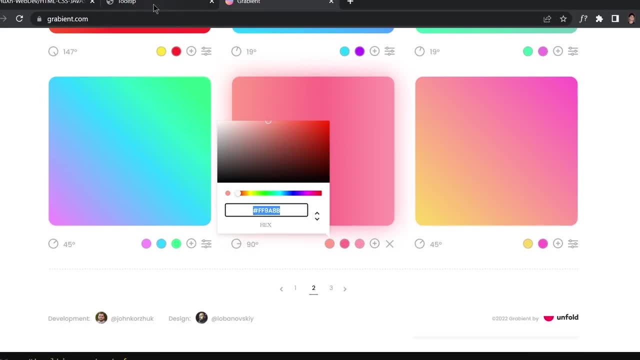 duplicate and comment this one. and now let me duplicate and comment this one. and now let me this line of code. and now let's change this one. and now let's grab the second one from there, copy it, and now let's change it to this one, and then, finally, we have this one. so let's copy this. 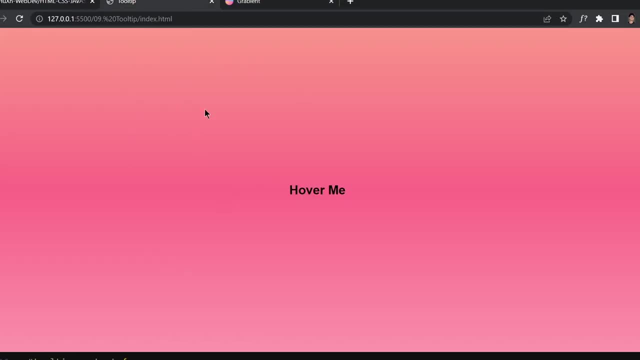 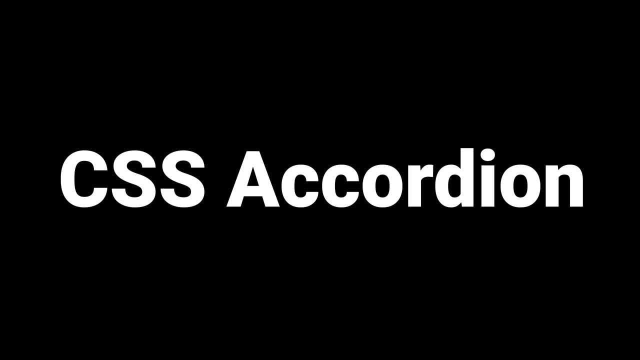 code and save our file, and now here you can see that background is changed. so i don't like that. if you like this, you can choose whichever gradient you like, and here's my gradient. hey guys, hussein and welcome to the 10th project of this course. so in this video, 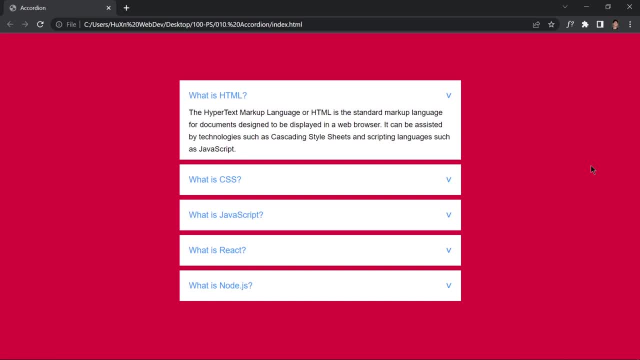 we are going to be creating this accordion's component by just using html and css, no javascript, no, nothing. so if you just click on this one accordion, so it will collapse the above and it will open this one. that's because we are going to be toggling or active class, so you are. 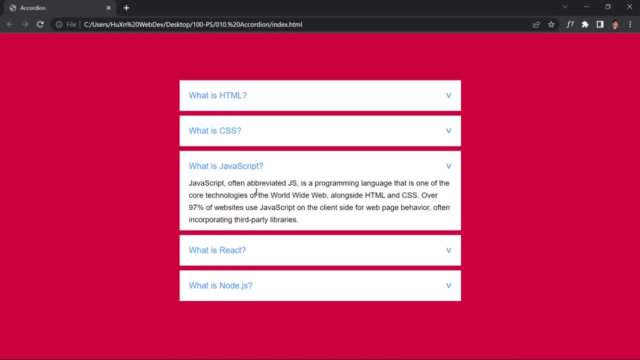 going to see that just in a second. so if you click on this one, so it will hide this one and we'll open this one, okay, so this is how it looks like. so, without wasting any time, now let's jump right into our quarter and write our code and in the priest, where we've created this tooltip by: 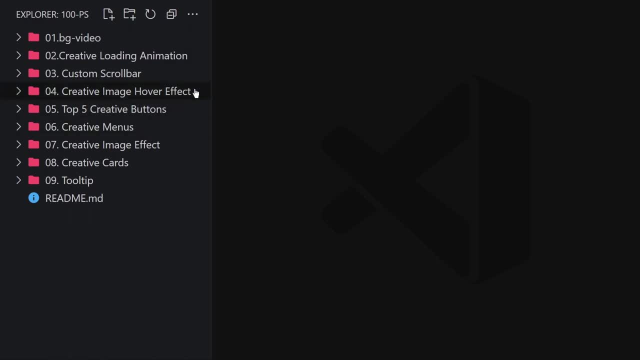 just using html and css. in this video we are going to be creating an accordion component by just using html and css. no javascript, no css, preprocessors like sas and etc. but just html and css. so later on in this course we are going to be also creating an accordion component by using 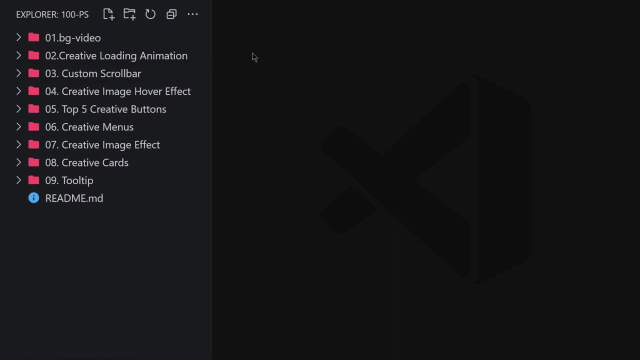 html, css and javascript, but in this specific video, we are going to be just building it by just using html and css. so, starting from the first thing, which is our 10 project, and now we have to do, we have to give a name of like accordion, and now head in here, inside this folder, i want to create: 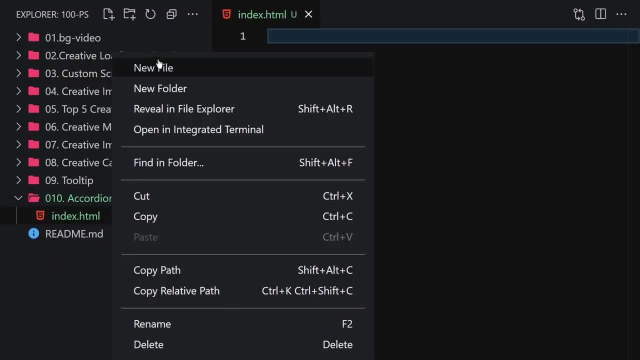 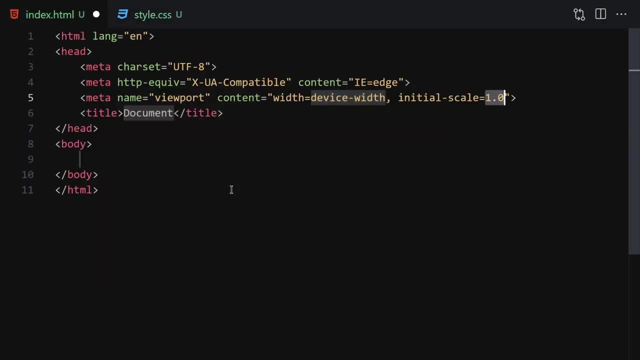 two files. the first one will be indexhtml and the second one will be style stylecss file. so now let's try to html code. so i'm going to write doc type html, and here i'll just give a name of, like accordion, and now just link it with css. okay, so, so now let's open it in our live server. so i'm 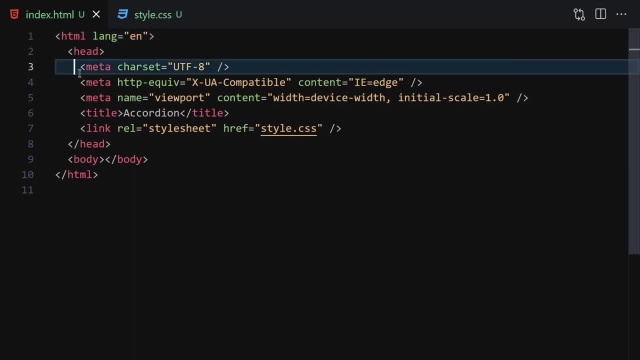 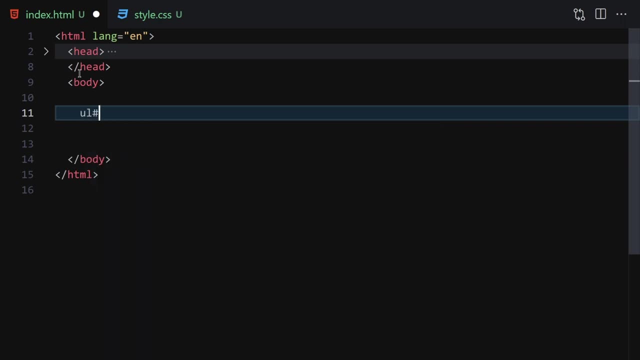 going to just right click on it and go with live, and now let's collapse this metadata as well. okay, so the first thing which you have to do is that we have to just write a ul with the id of accordion. okay, inside this ul, we are going to be writing our li. inside this li, we are going to be 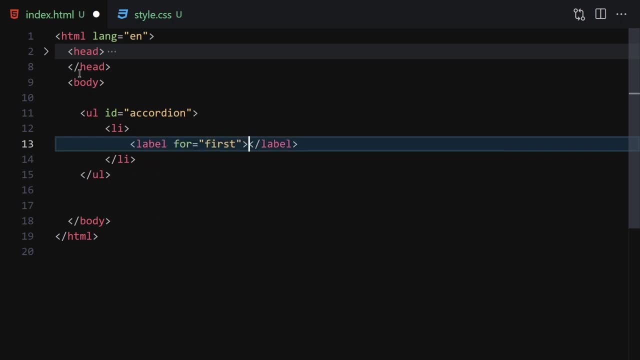 writing our label and the first four we are going to be writing a first and one is html. you can put whatever question you like and then we are going to be writing our span right here and then here we are going to be using an html entity. so if you guys don't know about html entity, you will just 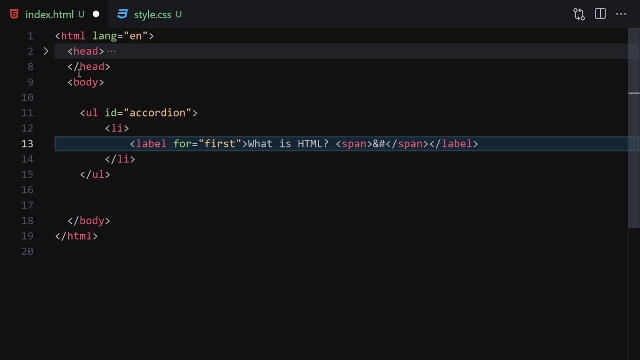 need to do this. first thing which you have to do is to just write an and symbol, then pound symbol, then write x, and then three, nine, then three e, to be precise, not nine. and now let's close it by just writing a column right there, and then the next thing underneath, uh, the label we have to just 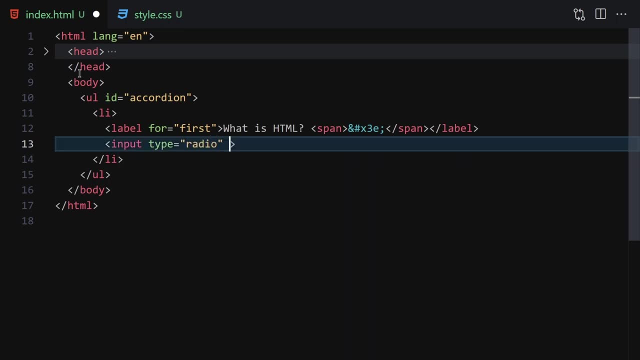 write an input and it will be a radio. and now let's give him a name of like accordion. and now the final thing which you have to do is to just provide an id to it. so i'll just give an id of first, and then we have to provide an attribute of check. 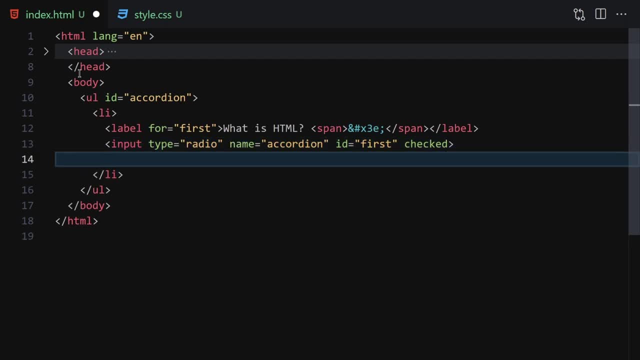 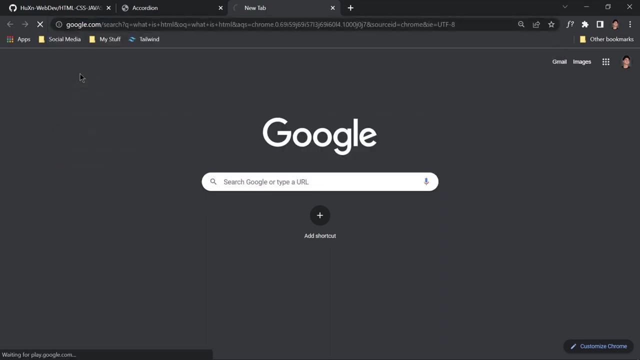 and this will just go for the first one of all of them. underneath this input box, we have to also create a div with the class of content, okay, and then here inside this content, we are going to be just writing like, uh, let me just go to, uh google and just search for, like, what is html? okay, so then, 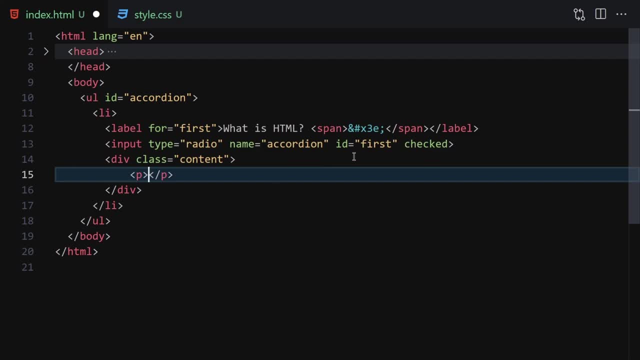 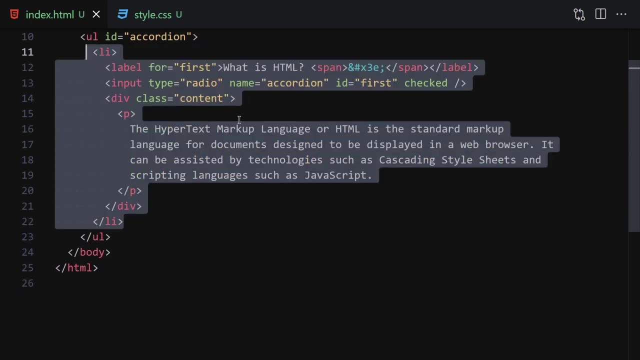 we have to just copy this text. you can just provide a lorem ipsum like a random text if you want to, but in my case i'm not going to go there, so i'll just duplicate a few times, like: what is html, what is, what is javascript, what is react and what is nodejs. so now let's change this text to like what. 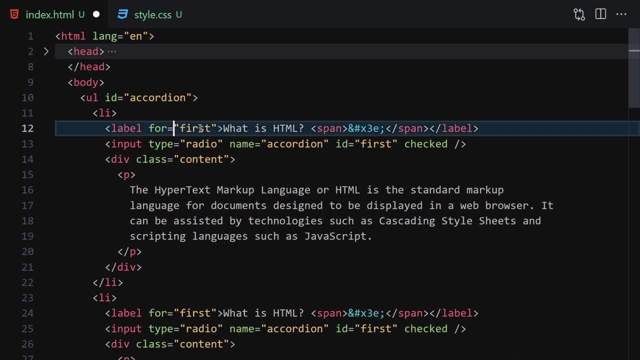 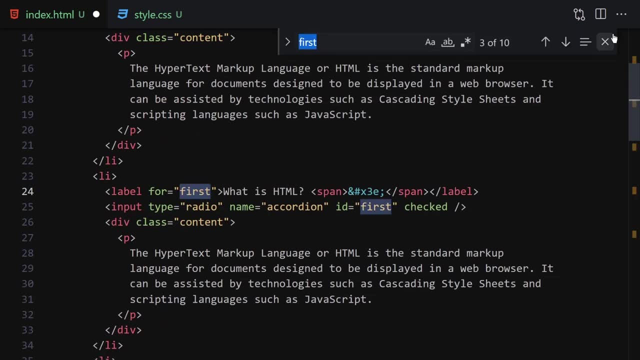 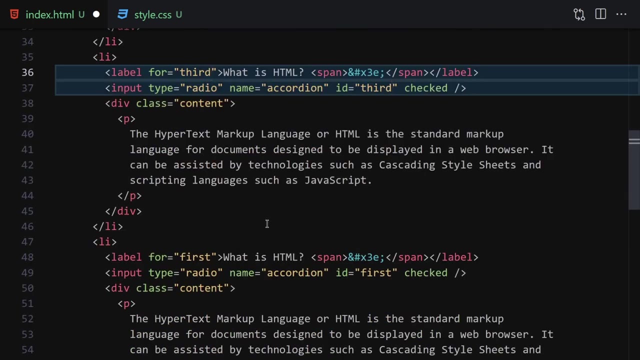 is: um, first of all, let's let me change these uh four and this already, so this one was first one and this one is now the second one, so just close that second, and then this one is third, and then this one is fourth and the final one we have is a fifth. 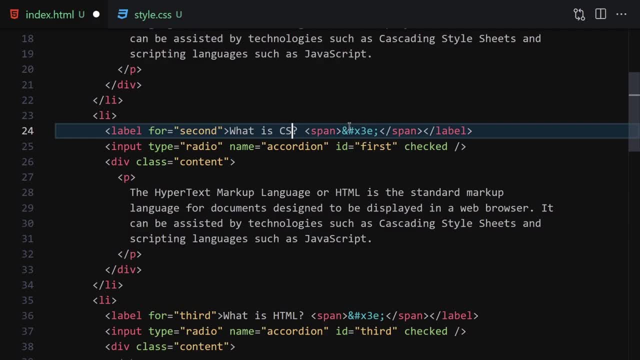 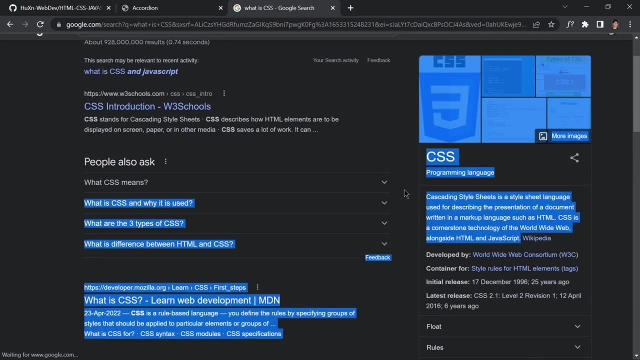 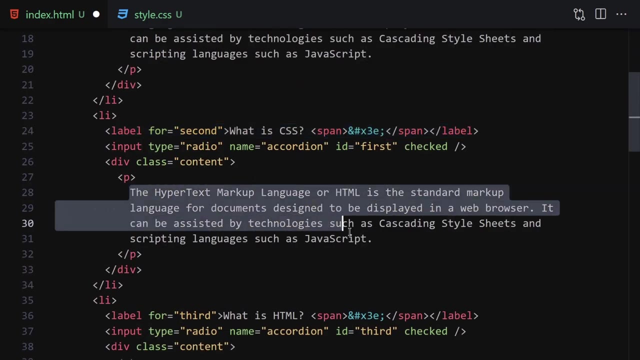 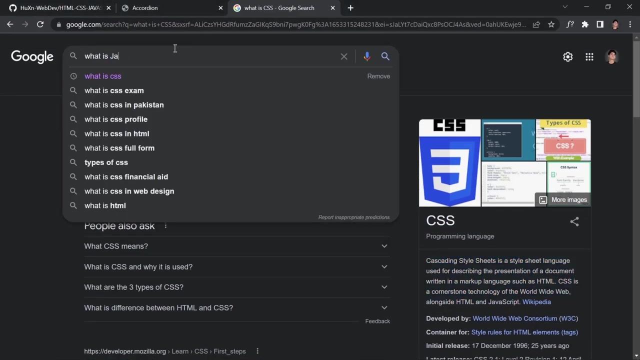 okay. so now let's change the text to: like what is css. and now let's ask google: like what is css? so apple gives us this result. now let me copy that from there to this place. and now let's just html: css, paste it right here. what is, uh, javascript, uh, javascript. 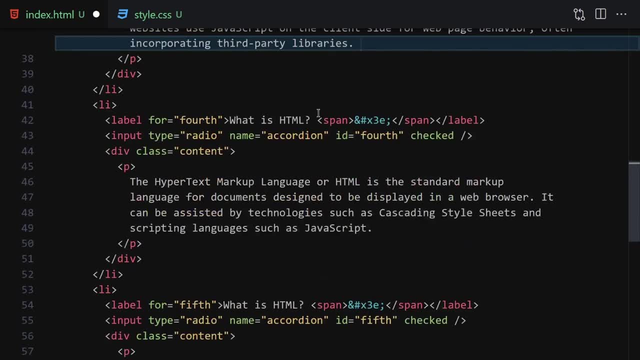 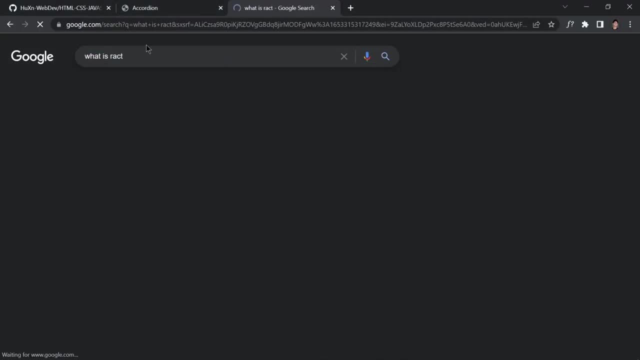 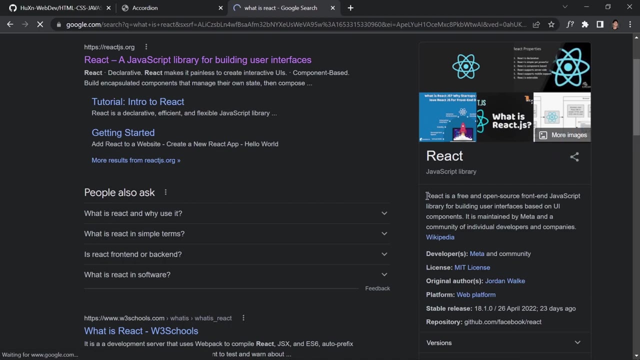 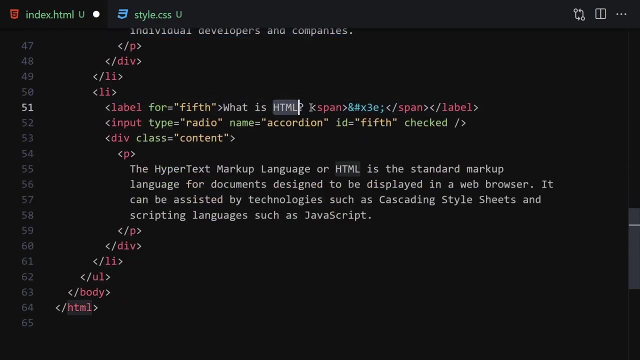 hold short. and now let's paste this text right here. and then word is: react, our reactjs, sir. oh, come on, mess, build, copy this text and i'm going to paste it right here. and then, finally, what is nodejs? so let's ask google, like what is? 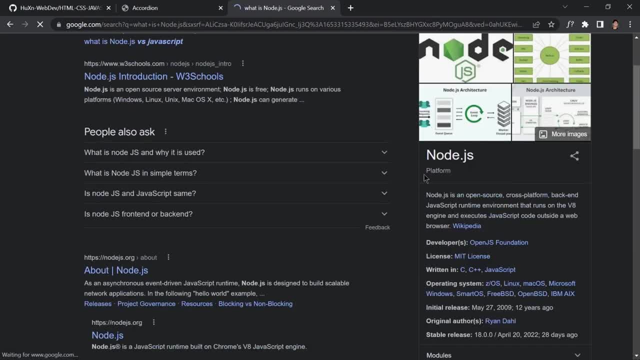 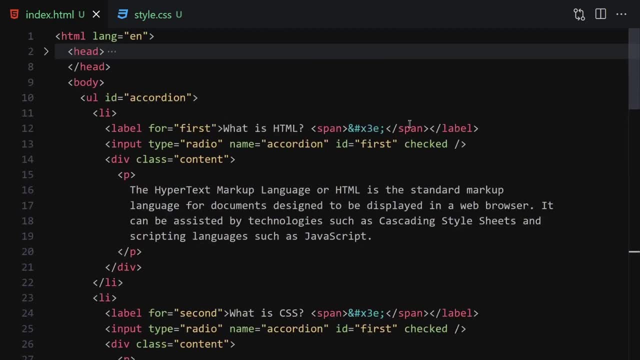 nodejs, so it will use this result- and nodejs is an open source, cross platform, etc. and then we will paste that here. all right, so now we are good to go. so we've changed the ids and we have to change the names as well. now we shouldn't have to change the names, but we just have to change the for. 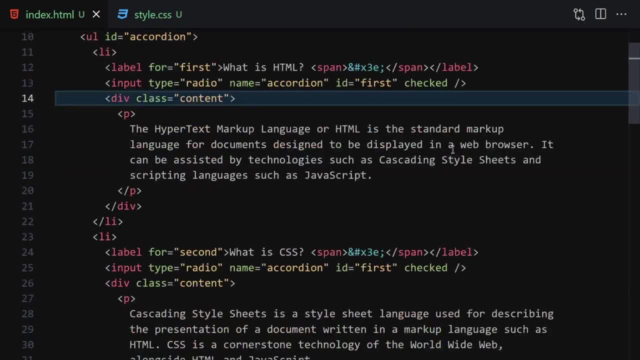 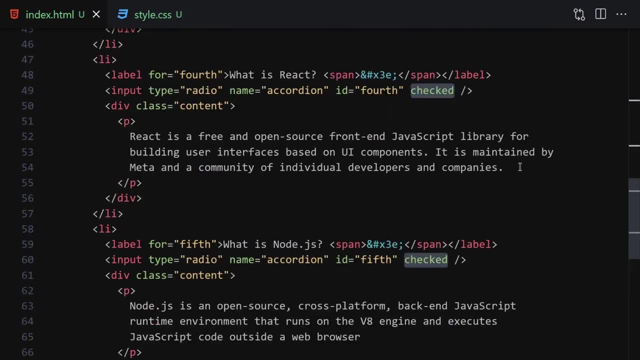 attribute and the id as well, and now we have to just remove this check from all of them except the first one. so i'm just select all of them except the first one, and now i'm going to remove it. okay, so this was it about html. so now let me zoom out a bit so that you guys can see everything. 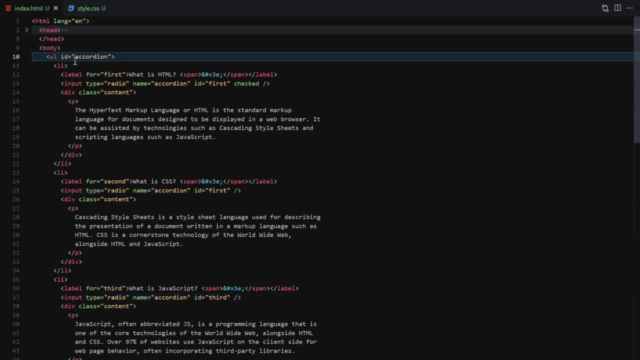 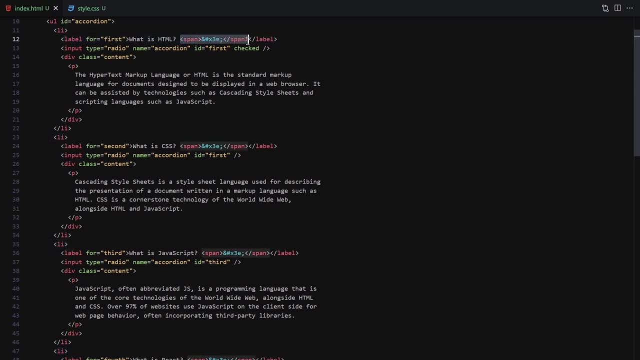 a bit clearer. so here you can see, we have a ul with the class of i, with the id of accordion, then we have a li, and then inside this li, we have a label, and then inside this label, we have this pen right here which will just show us this error right here. this is known as a error, but this is. 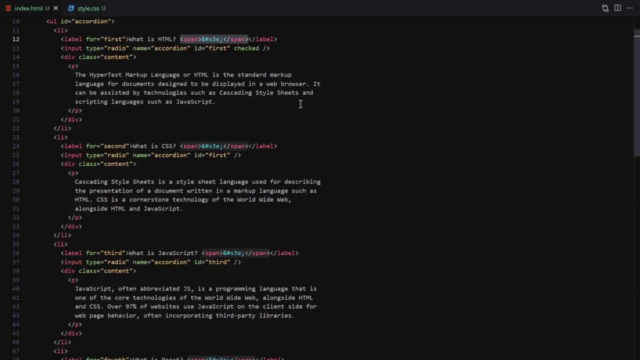 coming from html entity. okay, so if you search for html entity, so there is a lot of symbols you can use that you shouldn't have to, just like. you shouldn't have to just like copy the library, like font awesome or there's a lot of them, so you can also choose this icon if 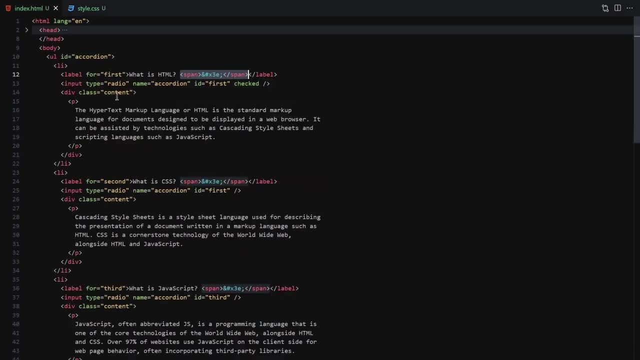 you want to. so then we have a content- uh- container. inside this content container, we have this paragraph which will just render these texts right here. okay, so now let me zoom in back and now let's jump right into our css and just start from the research. okay, so i'm gonna just write: 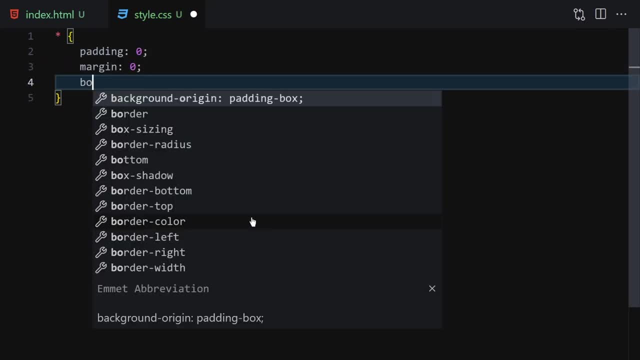 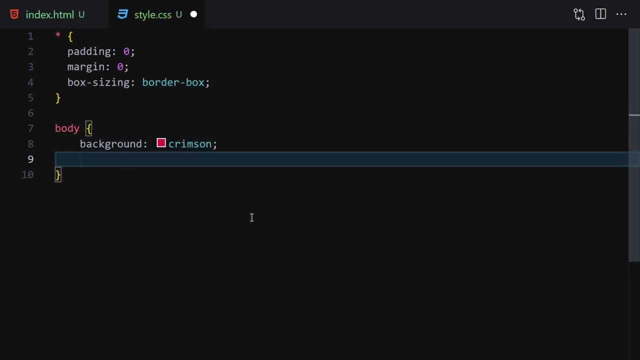 like padding of zero, margin of also zero and box sizing of quarter box. and now let's select our body. and now background will be crimson. you can choose whichever color or whichever um font you like. my guess i'll just go with the background color of crimson and font. 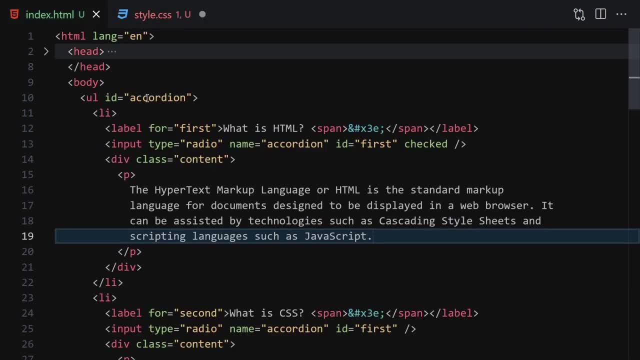 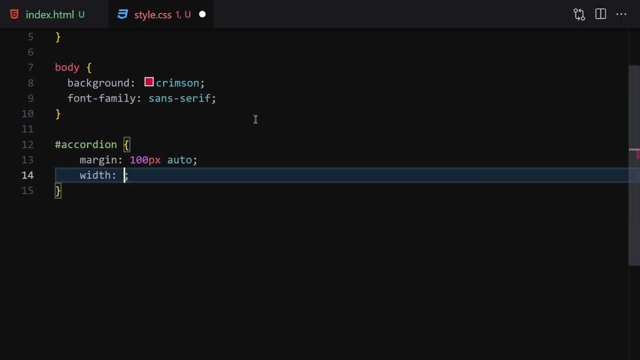 family of seven serif. and now let's select that accordion, which is right here and now. let's put a margin of 100 pixel and auto, and the width will be just 600 pixels. so once we save it- and this is how it looks like currently, right now- okay, so now let's select our accordion. 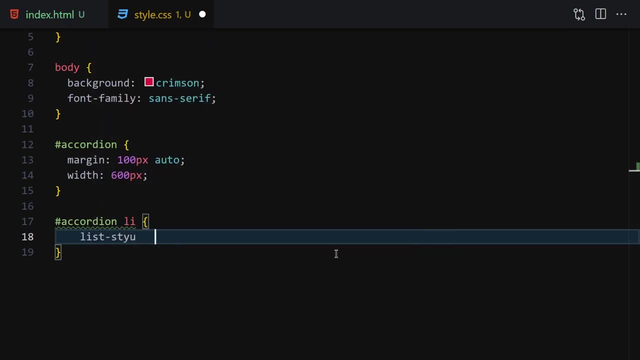 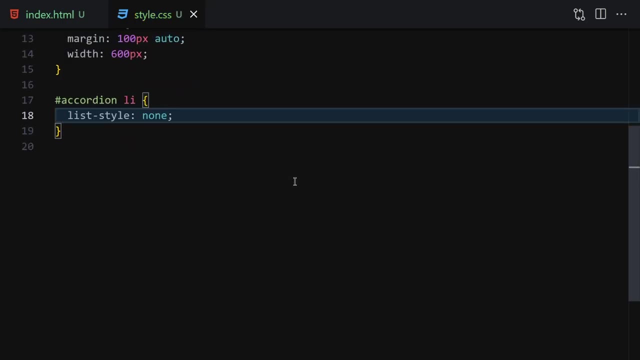 and also li. so now we have to provide a list: style of none, style of none, because we want to just remove those uh styles. and now let's just uh format a bit. so i'll provide a width of 100 and i'll just put a margin bottom of 10 pixel and the background will be totally pure white. 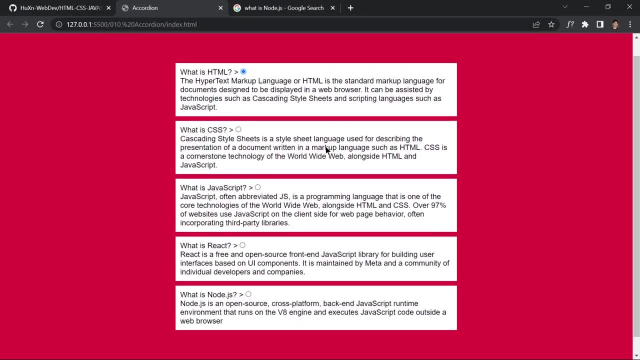 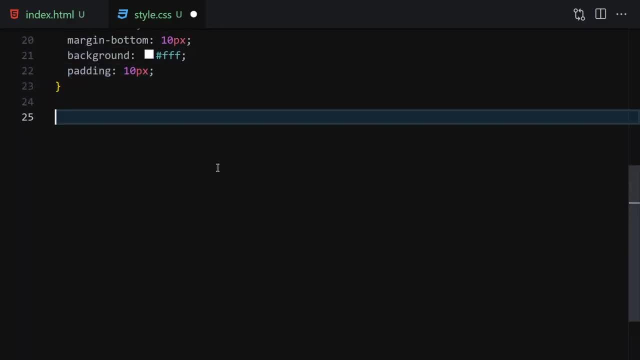 and padding will be 10 pixels, so save it and this is how it looks like currently. right now, so you have to just provide a bit of padding and setup right here. so now let's select that, or you know what? let me select all of that and paste it right here and 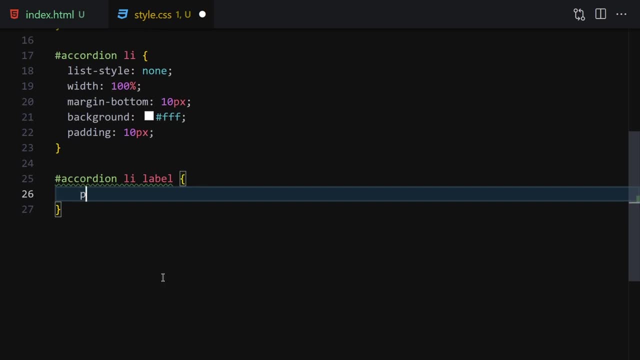 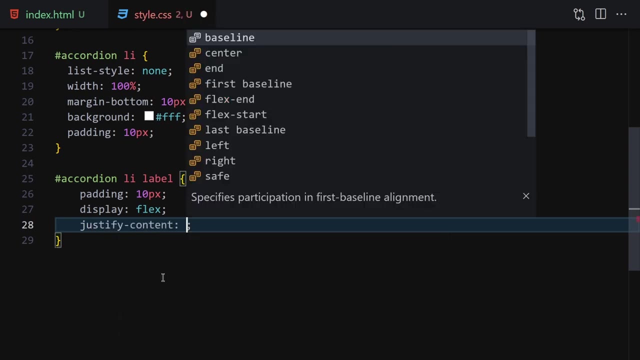 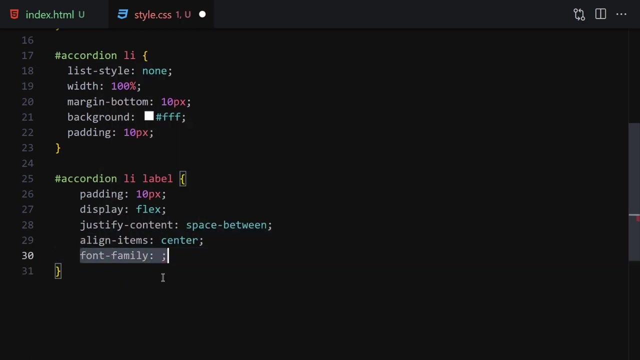 also select that label, and here i'm going to provide a padding of 10 pixel. all around display will be flex, justify content will be space between and align items will be center and font family- not font family, but uh, font size will be just a little bit bigger, like 18 pixel, and font weight. 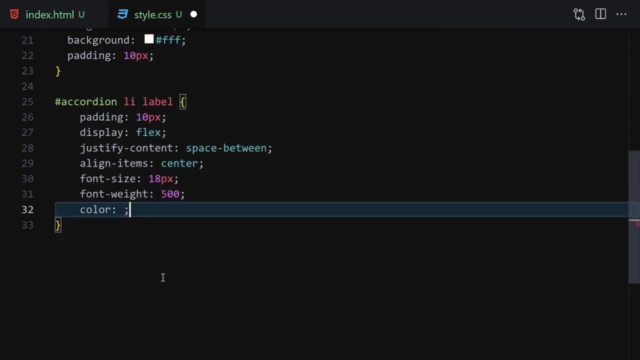 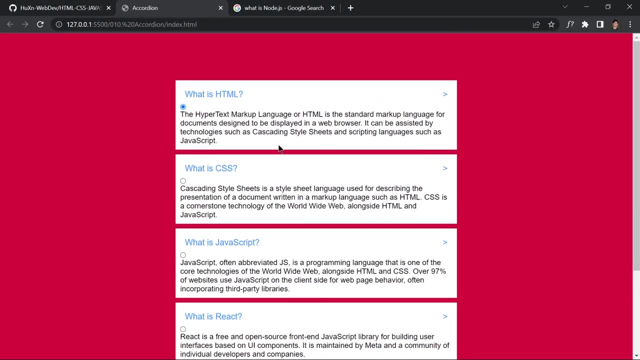 500 and we can change the color to like georgia blue, um dodger blue, or yeah, i guess that would be fine and cursor will be pointer. so once you save it- and this is how it looks like currently, right now, and we can also see these um this radio button right here. so now let's just remove that. 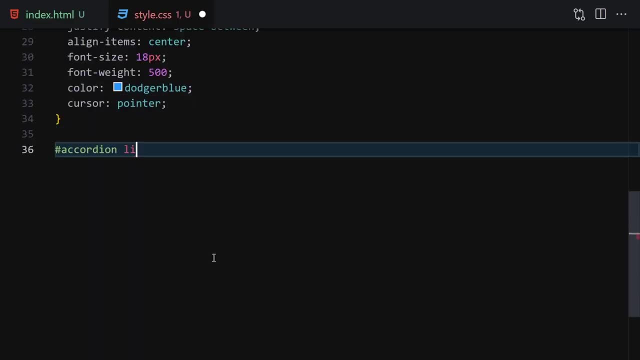 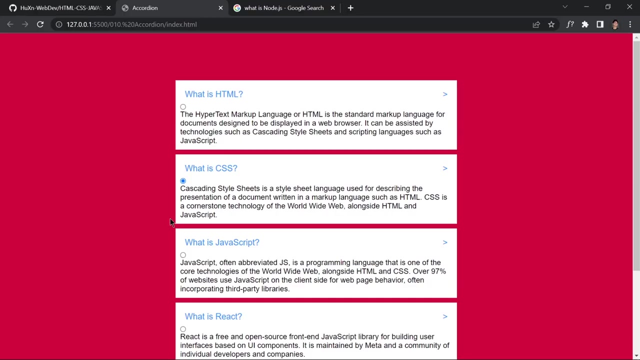 okay. so i'm going to select that first of all. i'm going to provide all of that and then label uh, or you know, plus input, with the type of radio, and we want to remove the display of none, save it. and that's not gone yet. something is wrong. we've got accordion, we've 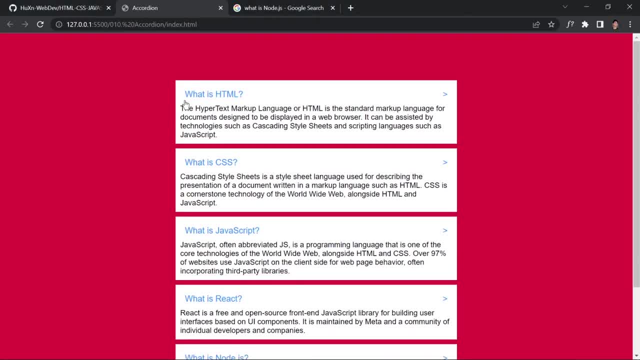 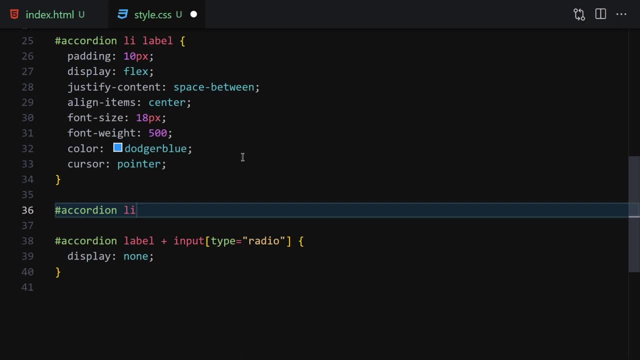 got a label label, save it and that is gone. now let's rotate this one to like 90 degrees so we can also do that by just writing like accordion and li, and then we have to just write like label and span, and now just prior transform of rotation a little bit like 90 degree would be fine. 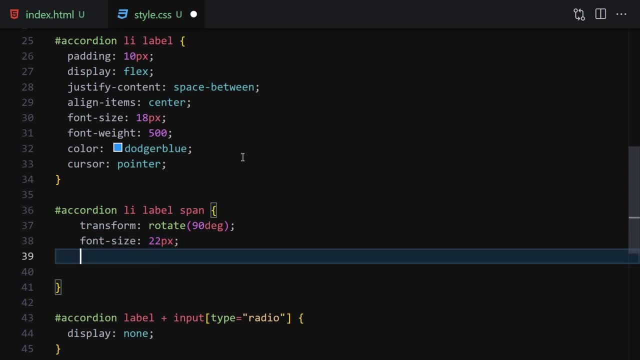 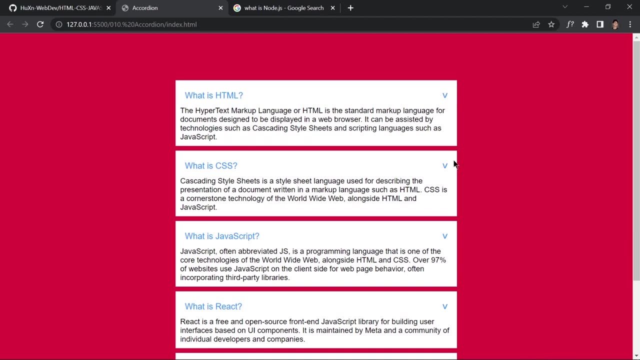 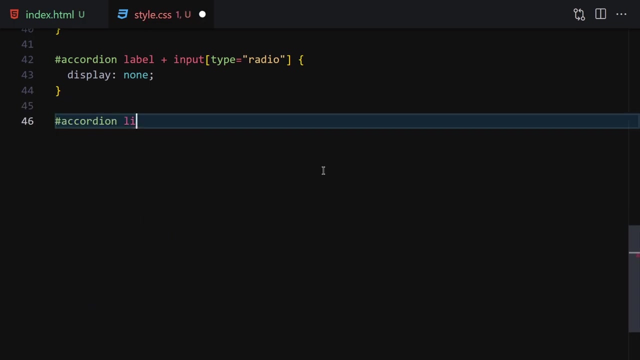 dec, and then the font size will be 22 pixel and then color will be that dojo blue, dodger blue, save it, and this is how it looks like right now. okay, so now let's just tile this text a bit, so that's that, and then we have to select this accordion. 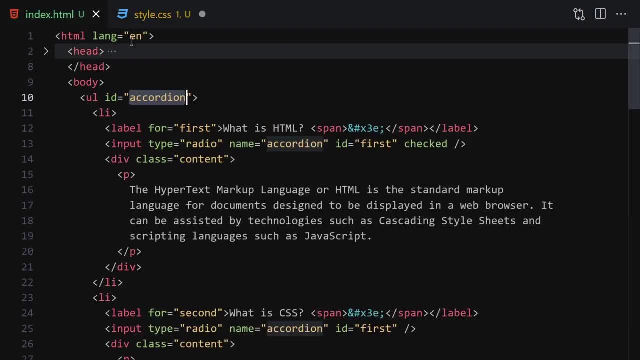 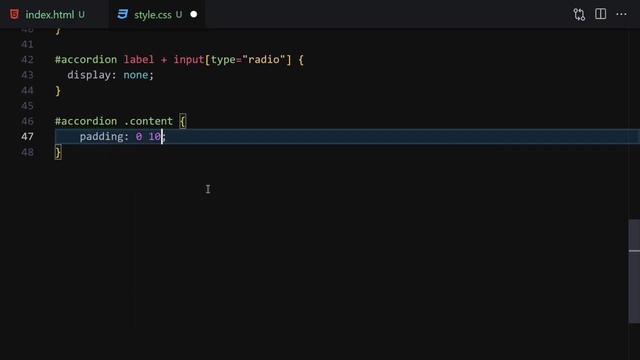 and now let's select that content which is right here. inside this content we have this paragraph. so now let's change that to: padding will be zero from top and bottom and uh til to left and right and line height will be just uh, 26 pixel, be fine, and then max height will be zero. 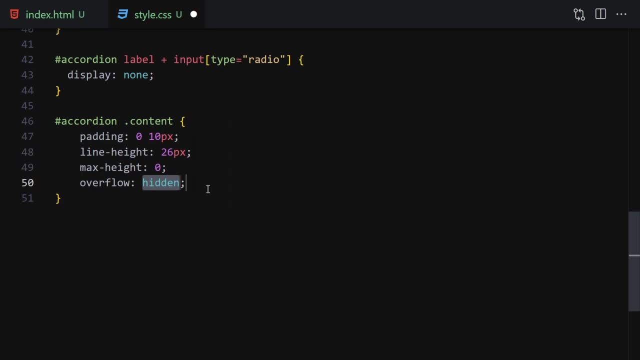 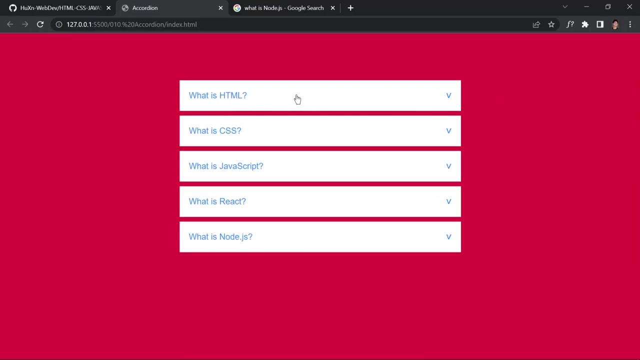 for now, because we want to increase that once we hover over to it or once we click on the button, and now we provide overflow of hidden and then the transition will be for max height and also from 0.5 seconds. so this is how it looks like right now. so once we click on this button or each accordion, 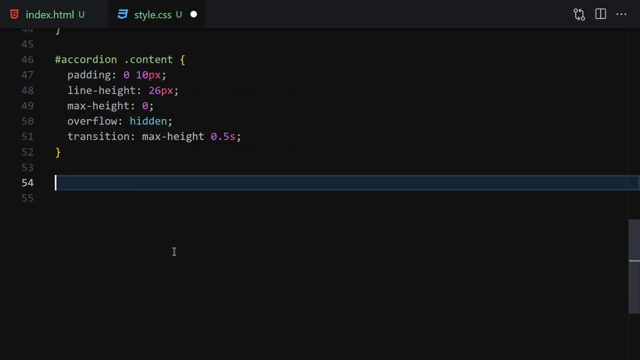 component, so you want to provide a little bit of max height to it. so this is what's going to happen right here. so now we select our label and then also or input with the type, okay, type of radio- and now let's select that, if that's checked, if some input is checked, so we want the content. 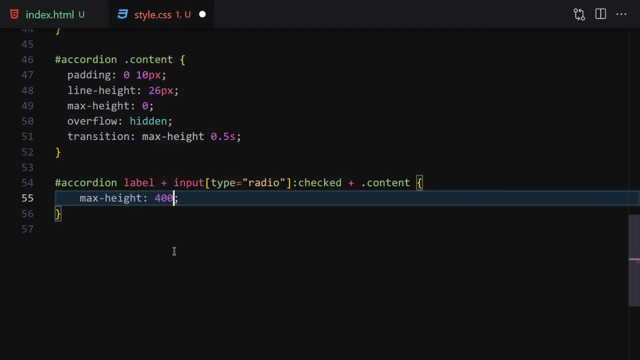 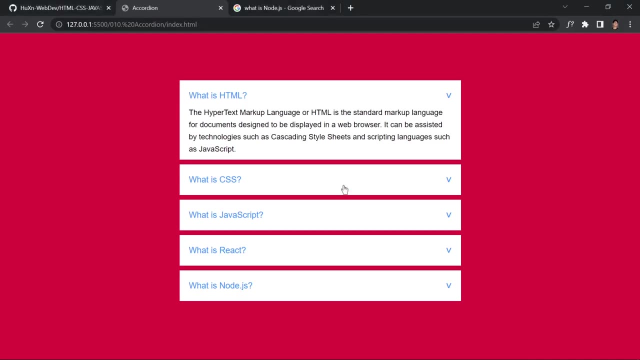 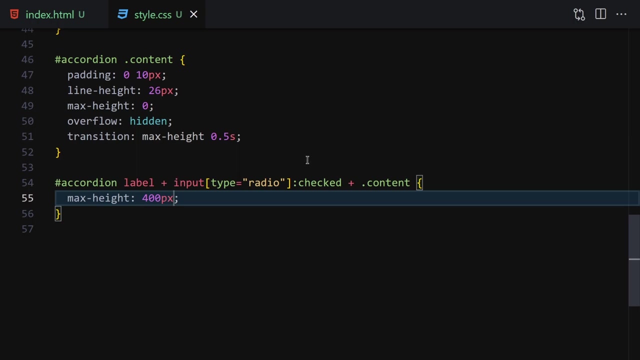 to just provide a max height of 400 pixels, save it. and let's suppose that first one was checked by here, so this one was checked. so let's suppose if i click on this one, okay, click on that one. now it's gonna happen. i don't know why. we've got our level, we've got our import, everything is fine, all right, so everything. 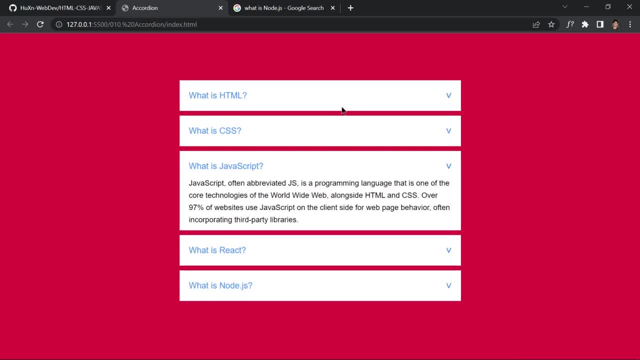 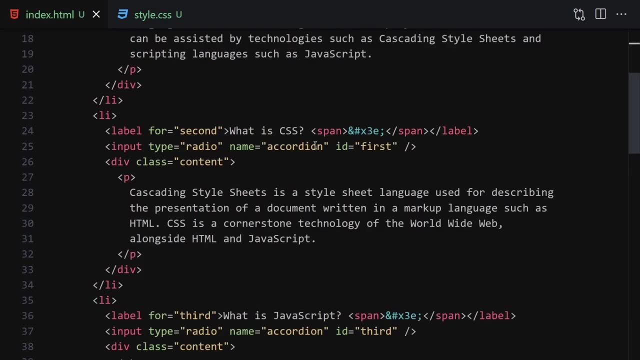 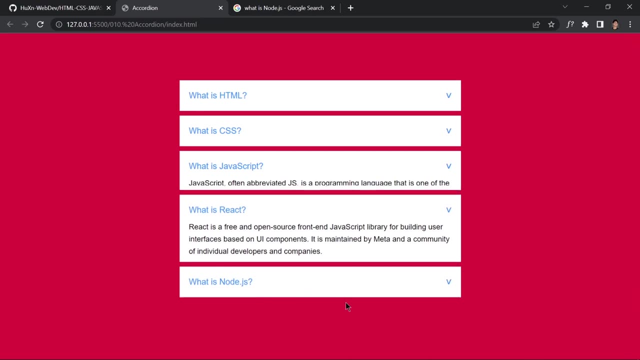 is working like this one is working. this one is working, everyone is working except this one. so i guess there will be a little bit mistake in the html code. so, second and second, yeah, save it, and now it should work. so if i click on that, yep, it's working. 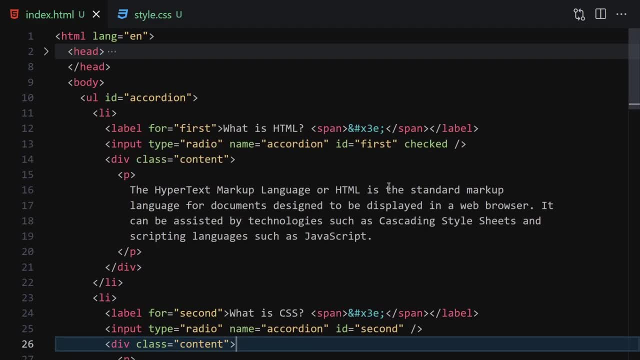 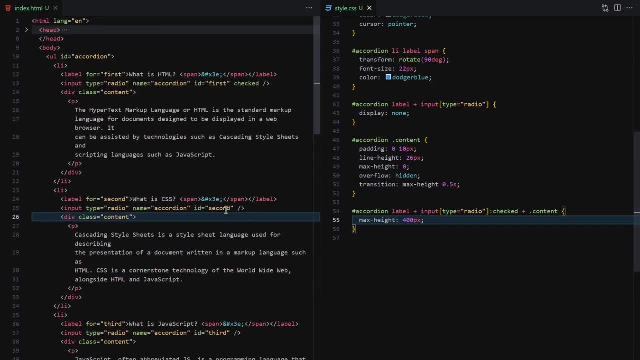 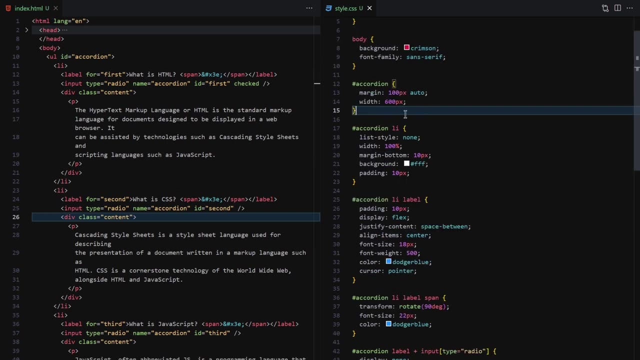 all right. so that was a little bit of html and css. so now let me zoom out a bit and show you both codes side by side and what we are doing. all right, so we are just providing a background color and font family and then we are just centering everything and we are just providing a little bit of width to it. 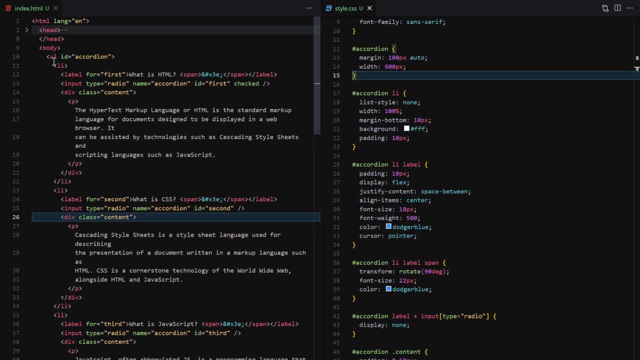 and then we are selecting that li, like which one are you? we are selecting that ally and we are just providing a list style of none and we are providing a hundred percent of width and we are just providing a margin bottom of 10 pixel and background will be totally wide and padding will. 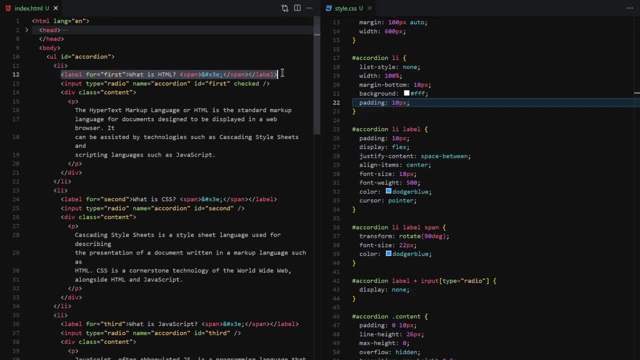 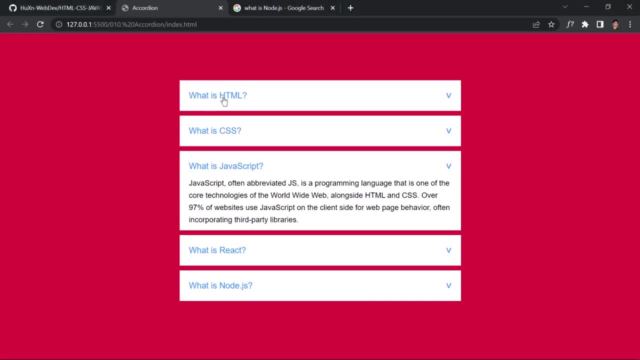 be just 10 pixel, then we are selecting that label which is right here, and then we have, we are providing like 10 pixel of label. we are centering everything, not centering, but just spacing around like this: one will take that plus and this arrow or html entity will take this place, and then we 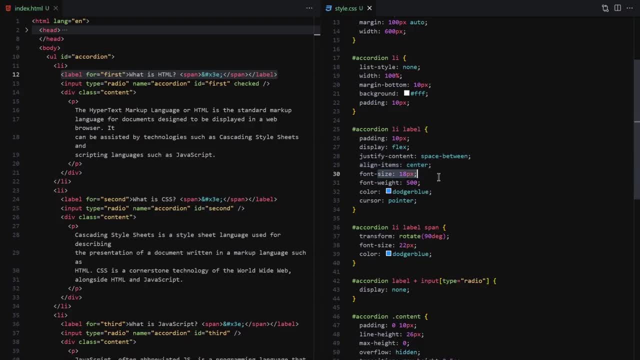 are centering in this component, and then we have a font size and then we provide a little bit of wear to it. we change the color to georgia blue, which here you can see that, and we just provide a cursor pointer to it, so like whenever we hover over to it, so that mouse cursor will be. 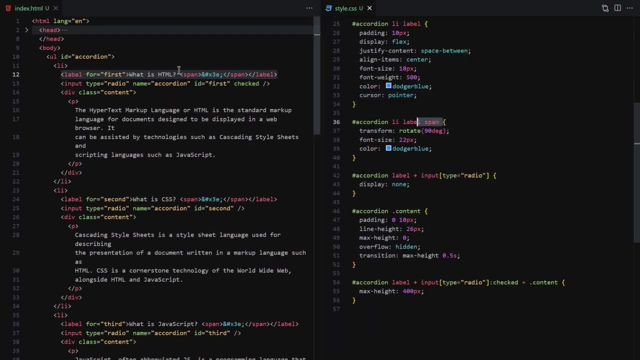 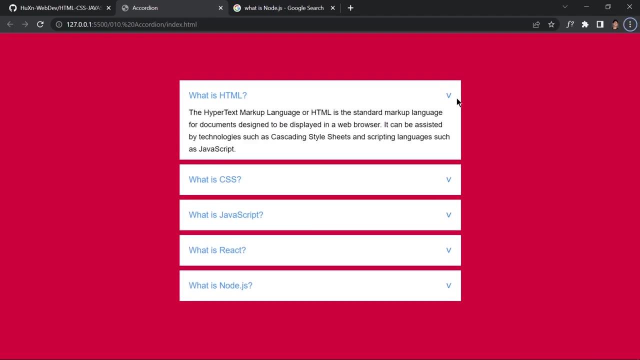 changed and then we have: uh, accordion, we select this pen, which is this pen right here, and we just rotate there like 90 degree. so here you can see, if i just remove that. so here you can see, this is going to look like that. and if i just rotate it, rotate it. so this is how it looks like, all right. 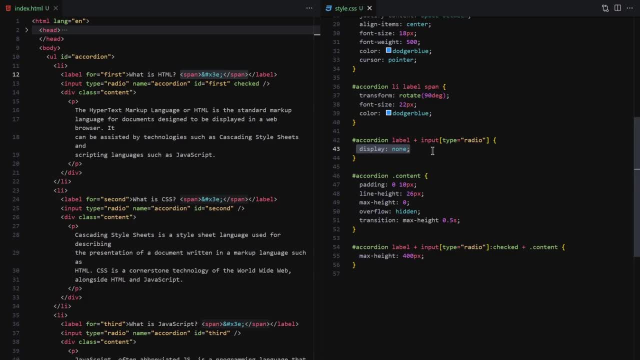 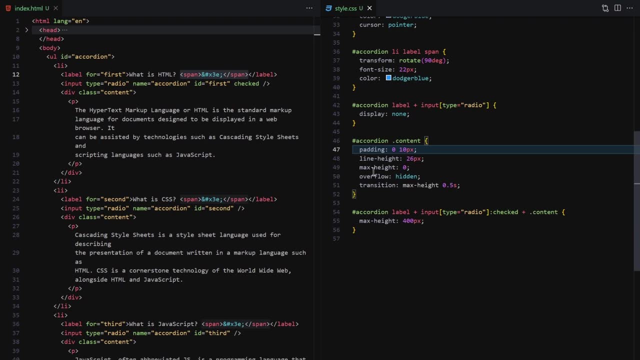 so then we just select our radio button and we just remove that display often, we just remove that radius from there and then we have our content. we are just providing padding and line height, max height and overflow of hidden and we are providing a transition of 0.5 second seconds on max height. so whenever we 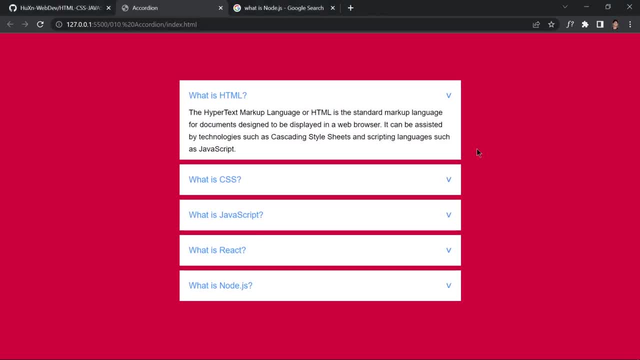 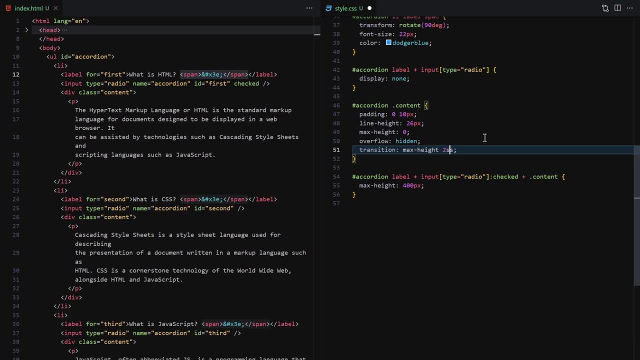 are providing a max height to it, so it will take like 0.5 seconds. so if i click on that, it will take 0.5 seconds. if i change this to like uh, i don't know- like maybe two seconds, save it. and now, if i 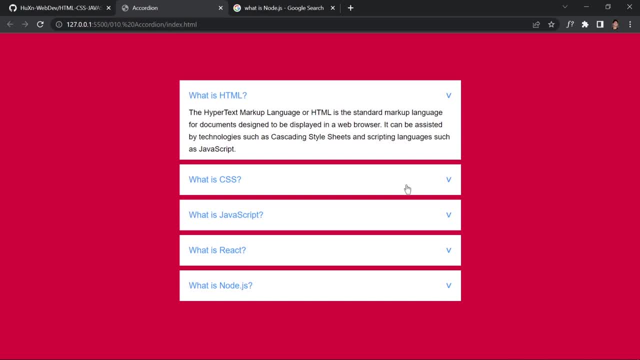 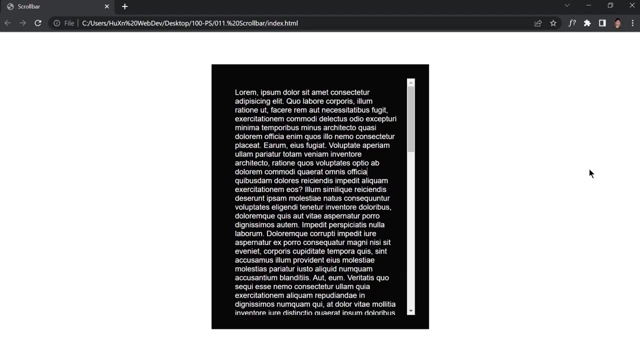 click on this accordion component, so it will take a little bit of time right here. so here you can see it's looking quite ugly, so maybe i should just go with 0.5, and now, if i click on that, everything is cool. hey guys, hussein, and welcome to 11th project of this course. so in this video we are going to 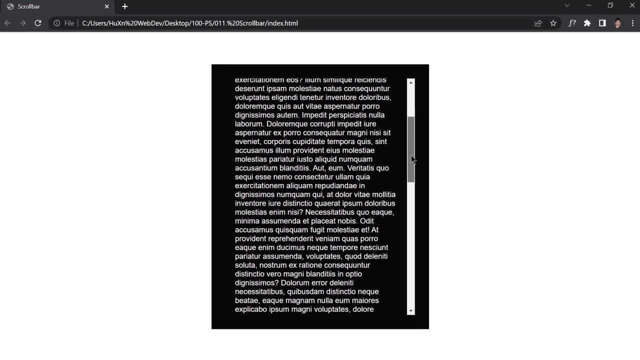 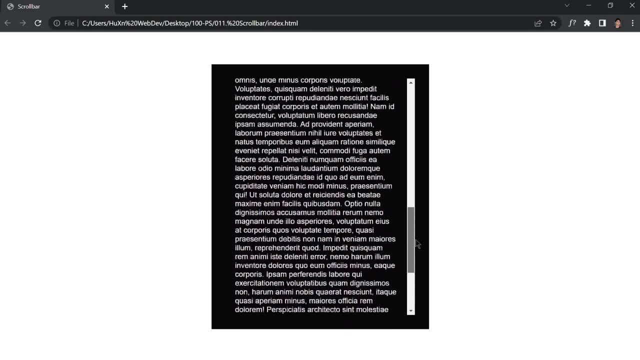 be creating this scroll bar by just using html and css. no java script, no, nothing. so a lot of people asked me about like how to create a scroll bar in our project. so this is what we are going to be doing in this video: by just using html and css. so, without wasting any further time, now let's. 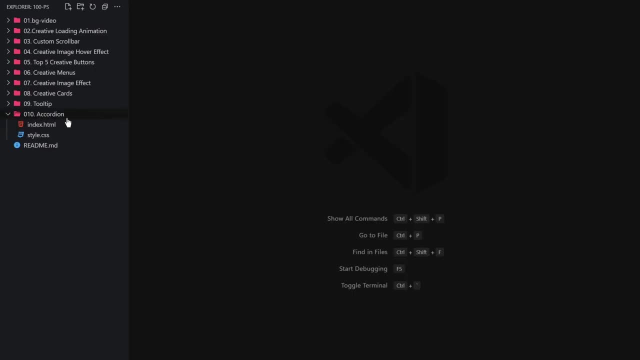 get into our code editor and write our code in the previous, where we've created this accordion component by just using html and css. in this video, we are going to be creating a scroll bar by just using html and css. all right, so i'm going to just write like: oh 11, and then okay. 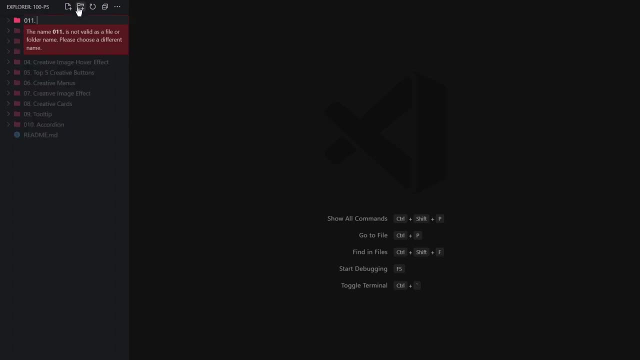 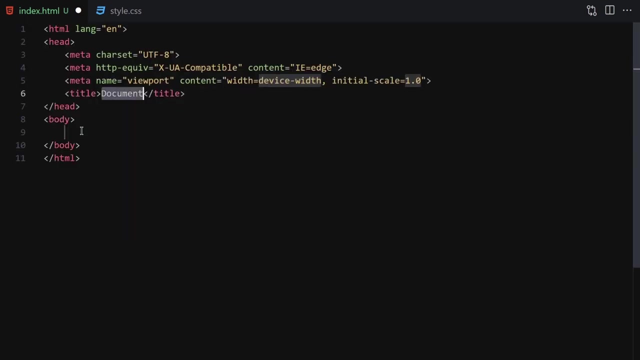 i should have have to give him some name, oh 11 and then scroll bar. inside this scroll bar folder i'm going to create two files given name of indexhtml and stylecss. this is minibird, so we can see it a bit clearly: doc, type html and then scroll bar and link it with my css. 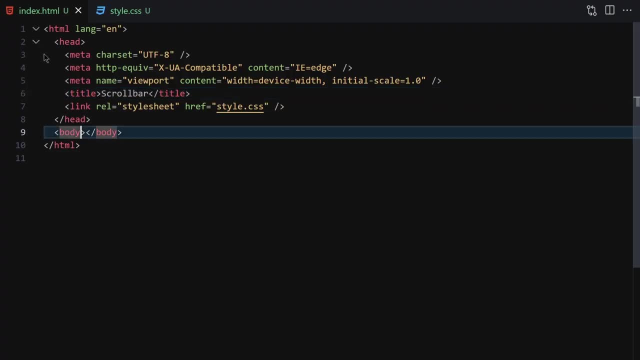 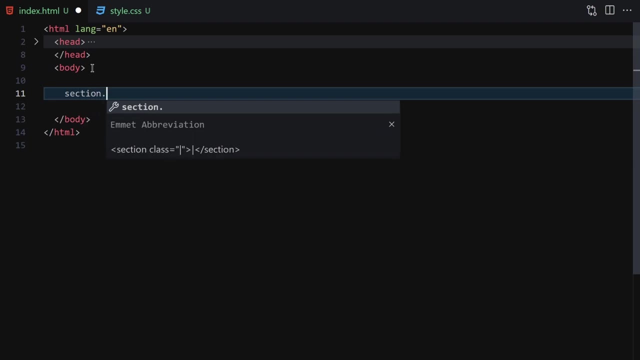 file right here. now. i'm going to right click on it and go live and also just hide this meta data for now. all right, so the first thing which i'm going to do is that i want to just create a section with the class of container, while you have a scroll live inside the scroll. 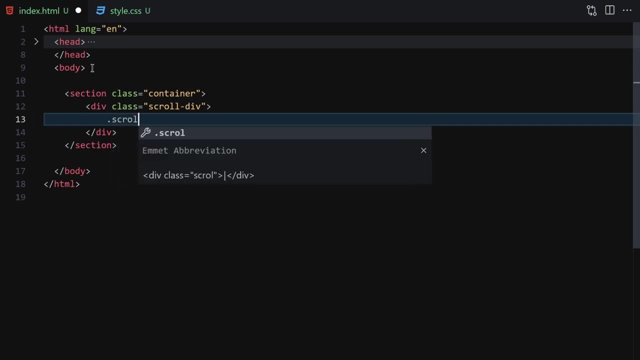 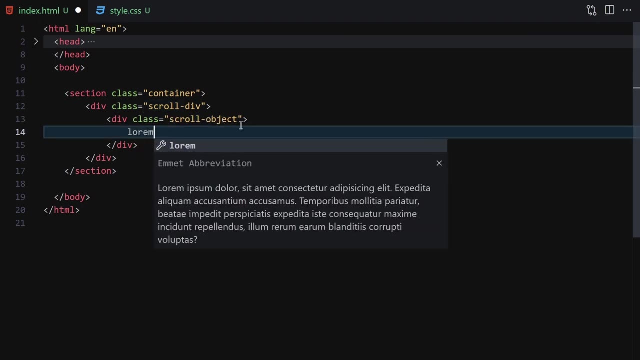 level. you have a scroll object, like a scroll dash object, okay, and here inside this scroll you're going to be writing a lot of text, so i'll just write like lorem of um. i don't know, maybe i'll just write like 500 texts and send my file so it will give us all of these texts. 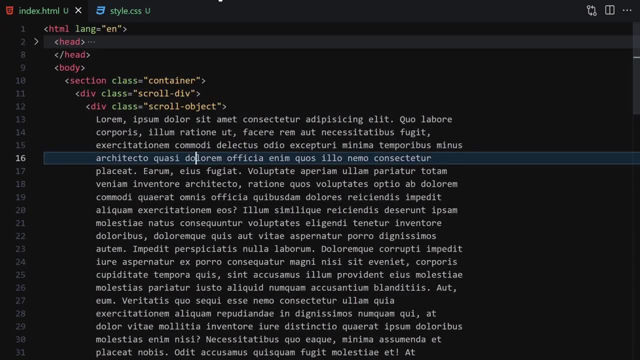 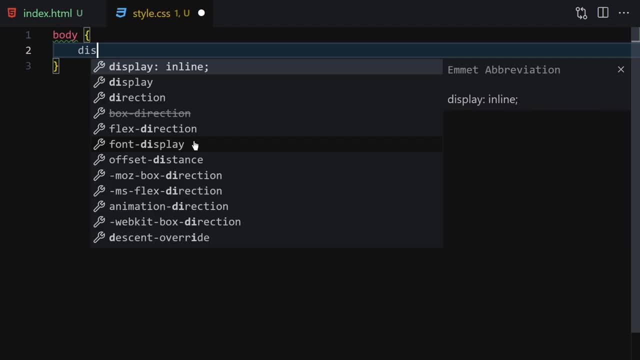 right here. okay, so this is quite simple and easy. so now let's jump right into our css and start styling. so the first thing i'll do is i'll just zoom in a bit and then select my body, and then the display will be flexed because we want everything to be centered. justify corner will be. 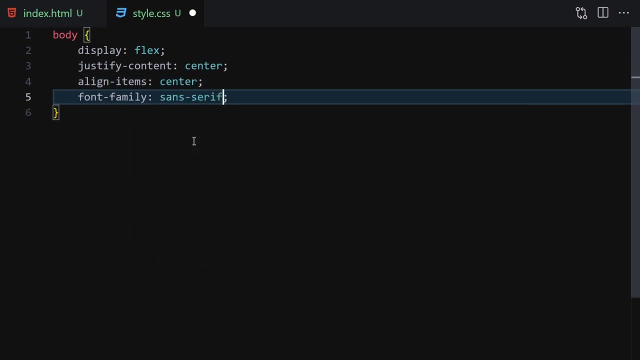 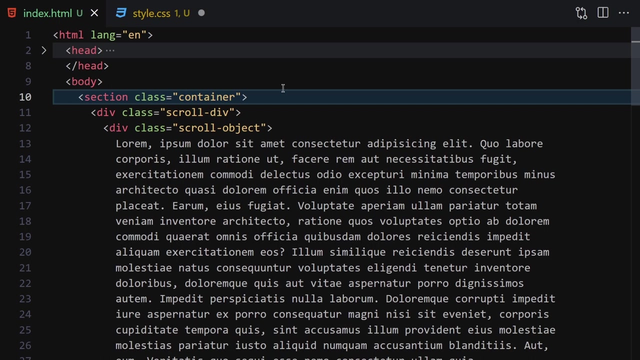 center online items will also be center font family. you can choose whichever you like, and so it'll be totally white. okay, and now we have to select this scroll container container, which is right here, this scroll container- okay, i forgot the name to like scroll container. so these are: 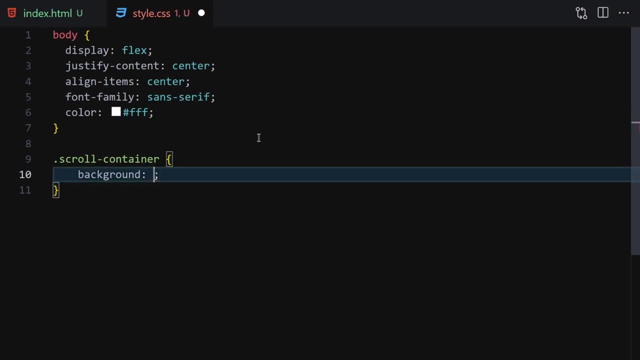 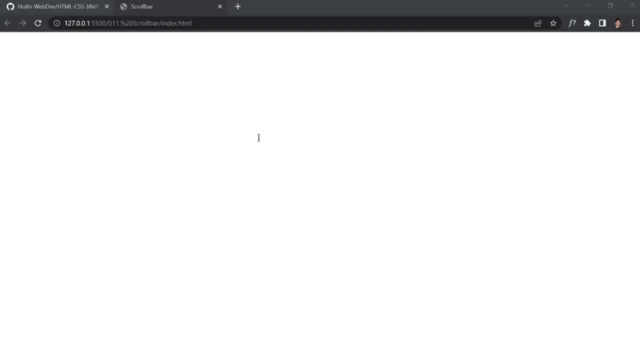 scroll containers. so now we have to give them a background color of uh rgb, and then the first one will be seven, seven, seven. and now we have to give them a width of 75, not 75- 25 around, and then padding will be 30 pixels once we save our file. so this is how it looks like right now. 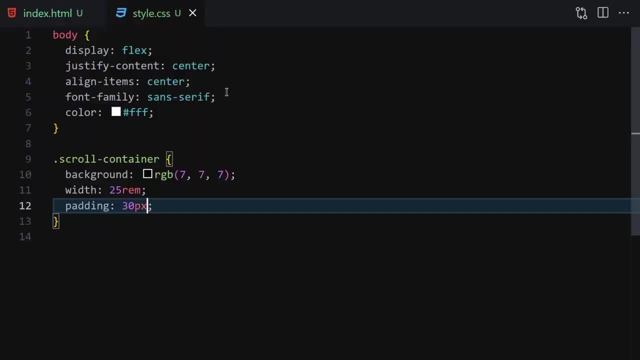 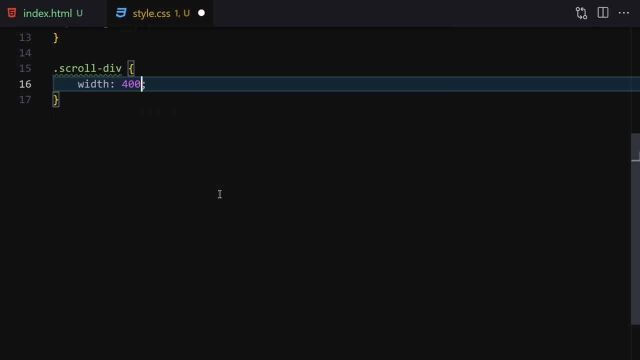 super, super ugly. okay, so now let's start work with this uh scroll div. so now we have to select that. let me just copy it. copy just a scroll div. and now let's select that scroll div right here. and now let's style it so width will be 400 pixel and height will be 500 pixel, and background color: 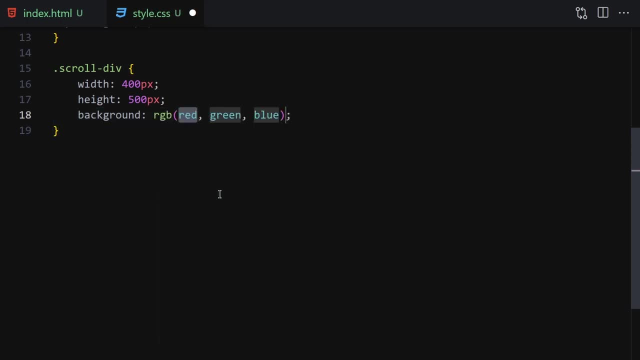 above. so rgb of seven, seven and seven, okay, and then we have to just provide an overflow, uh, of hidden, and then we have to just provide like overflow, um, of y, dash, y, and it will be scroll so once we save our file. so here you can see, now we get this scroll bar right here and we can scroll. 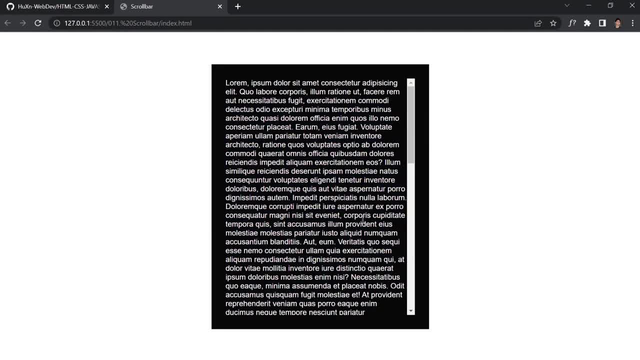 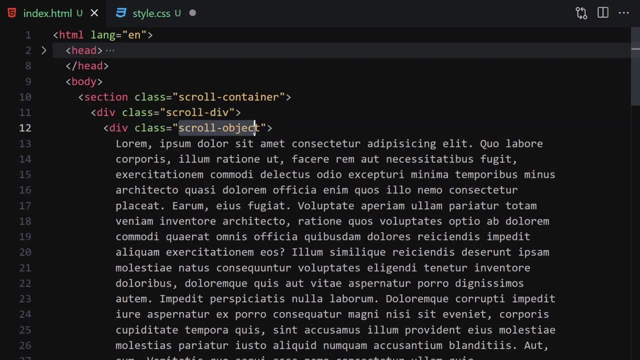 through right here. okay, this was quite simple and easy, and the last thing which we have to do is we have to just pour a little bit of padding to it. so i'll just select this scroll object and just copy it and then just write a dot and scroll object. 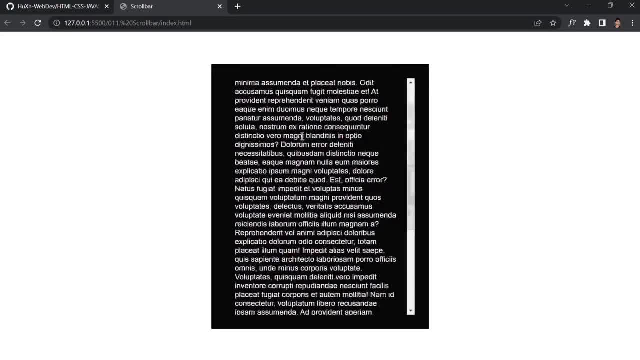 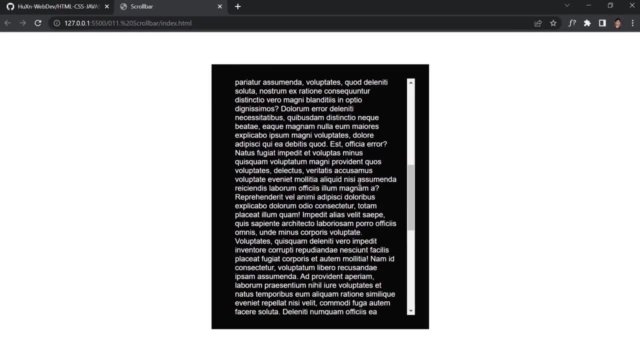 padding will be 20 pixels. save it. and now we got a little bit of padding right here so you can change the color. you can change whatever you want inside this project. but a lot of people dm me and tell me, like, how can we create a scroll bar? so that's why i'm 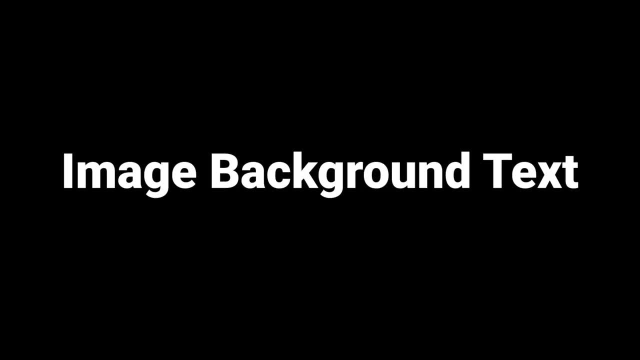 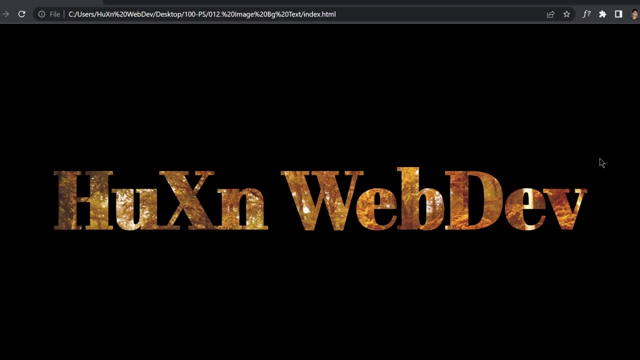 putting this project in my course. so there's that. guess who's saying: and welcome to a project 12 of this course. so in this video, we are going to be learning about how we can clip a background image as a text. so this is what we are going to be doing by just using html and css. no javascript, no. 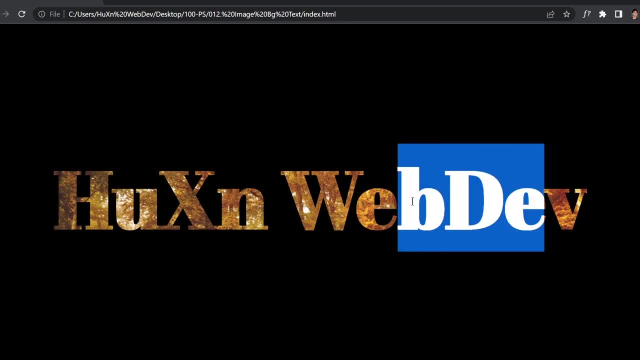 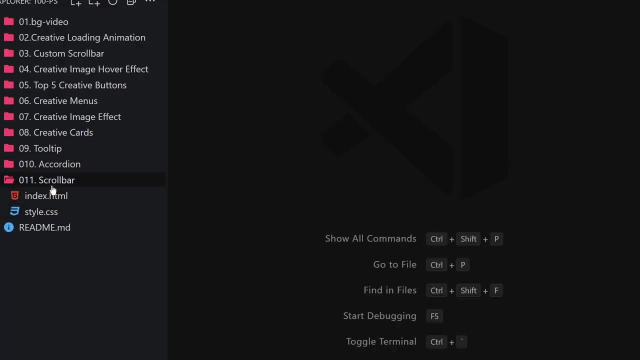 pre-processor? no, nothing. so, without wasting any time, now let's jump right into our coder and write our code in the previous, where we've created this callback component by just using html and css. in this video, we are going to be creating a background image clipper. 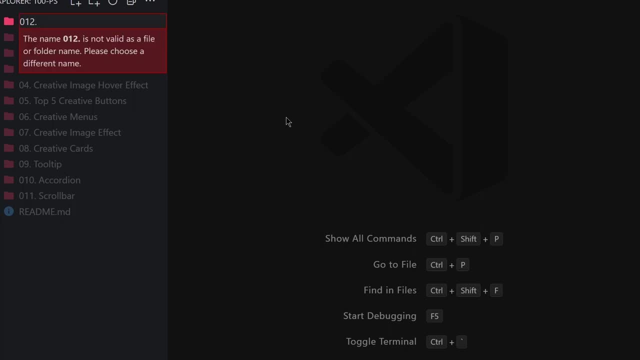 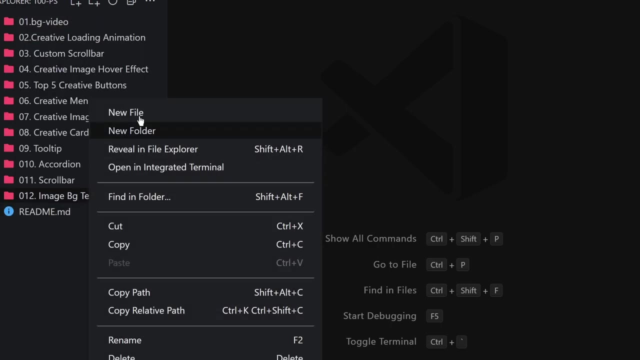 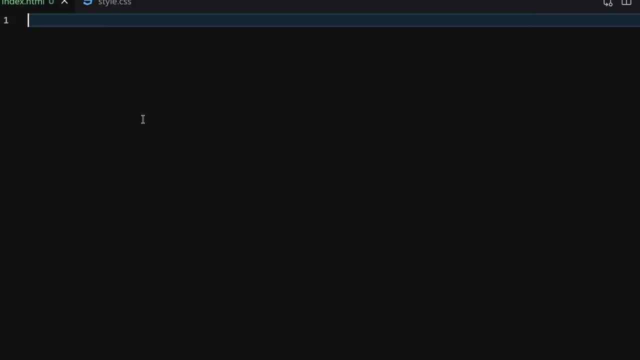 so i'll just write like code 12 and then i'll just write like image and then bg, or yeah, bg text will be fine. inside this folder i'm going to create two files given name of indexhtml and then stylecss. okay, then i'll just write my doc type html and then image, bg, bg text, and now 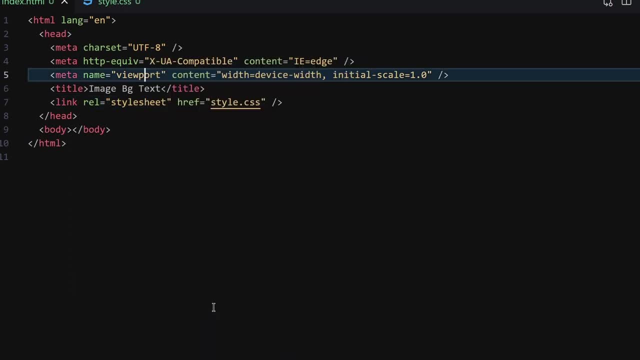 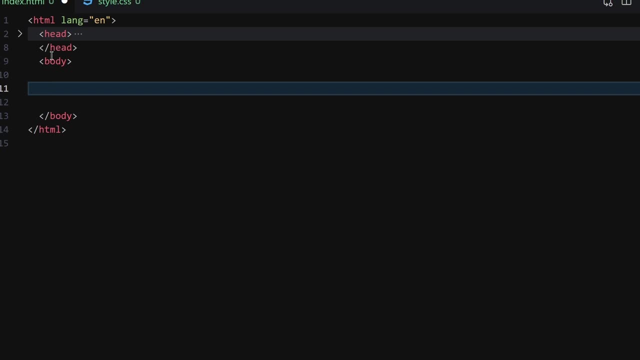 link it with css and then right click on it and open with live search. so everything is working the way we expect them to work, all right. so the first thing which i want to do is that i'll write a lot of html documentation and then i'll just write some other function like type, цвет and sorry. 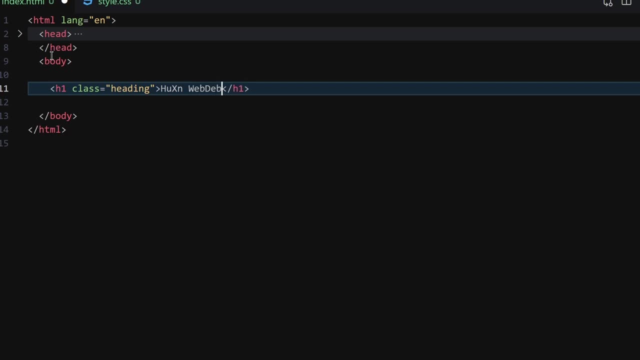 my settings here. so for example, i will write like html on website more stall exec and then create a layout name, kind ofnak and type of code list. then i'll already create a bothering html font save and i'm gonna save that too. and then this is a more standard version of. 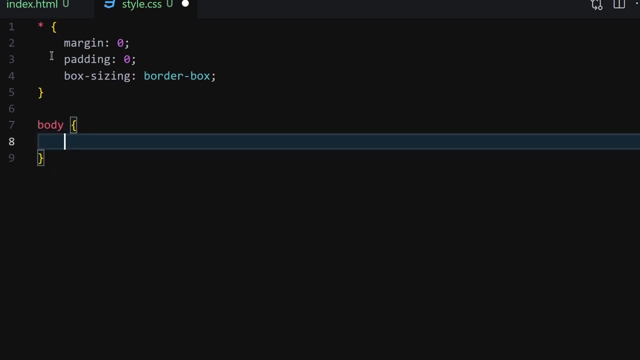 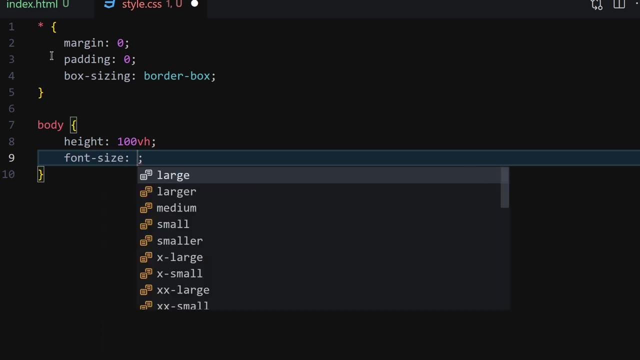 html for just heart, ficou, just write number right of 10, which is just right, like heading 100, vh. hired and font size will be i don't know, like um, i don't know. one rim will be fine. it's already by default one rim, so we have to just leave that there it is, and font family will be. 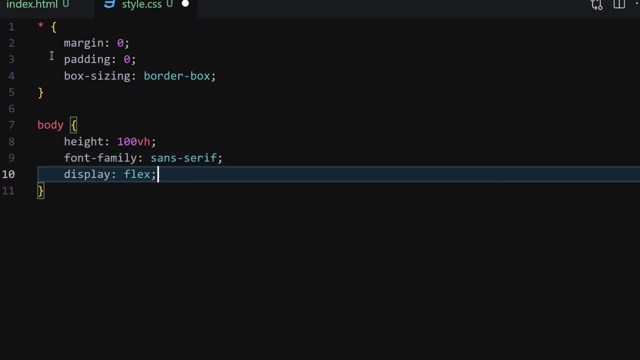 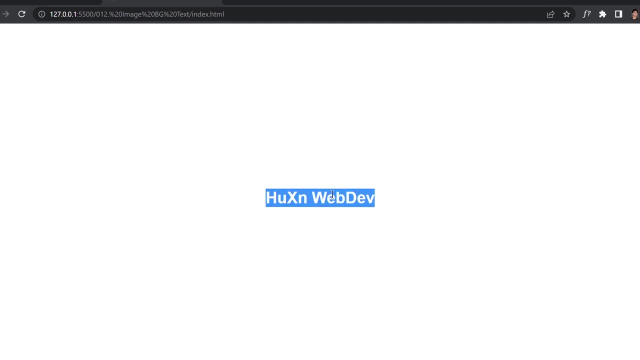 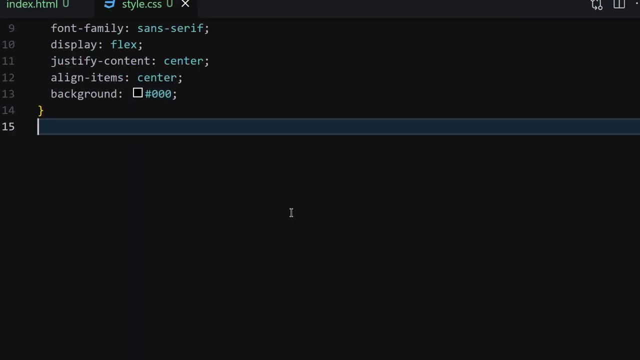 and display will be blacks, because we want them to be centered, and a light item will be also centered. okay, so this is our text and no breakdown whatsoever. so now let's just provide a background color of totally black, so i guess that was going to be looking a bit cool. and then, instead of 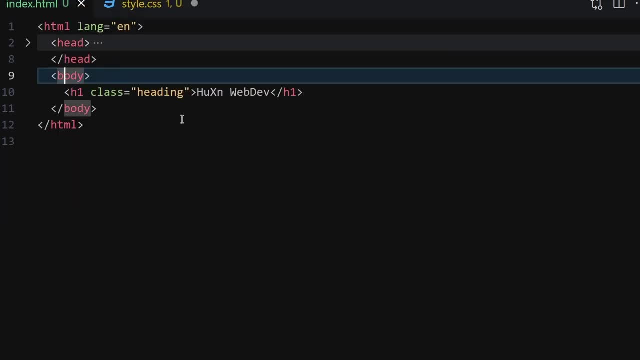 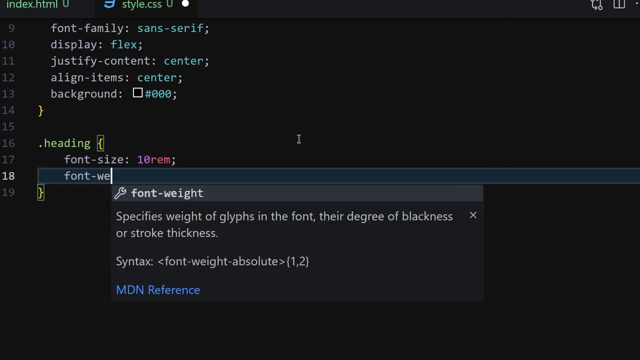 providing any colors. you're going to be just selecting for heading, which is right here and now. we have to just provide a bit of styling, like: font size will be 10, rim and then font weight will be 900, or yeah, i guess i'll go to 900, and then background image. let's grab a background image. 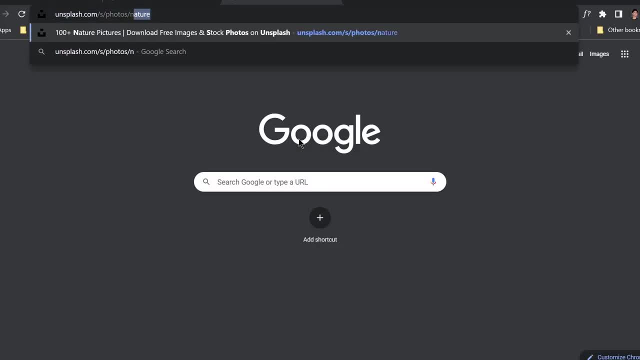 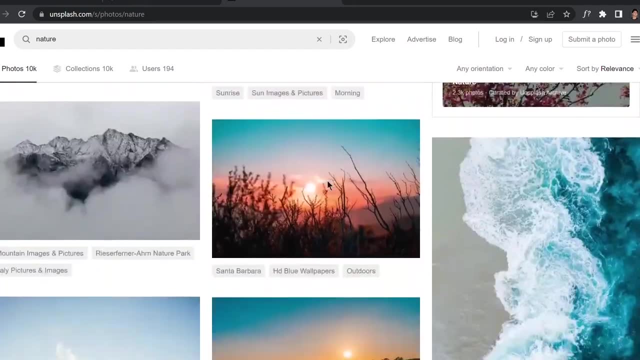 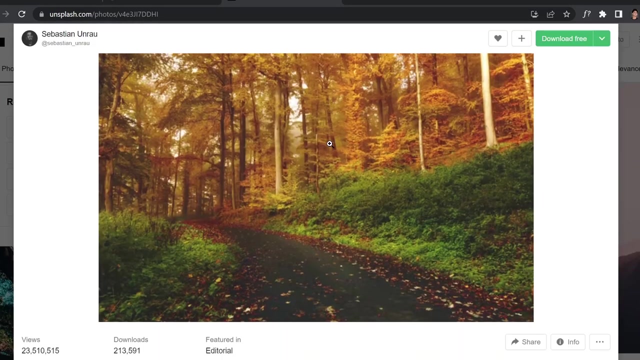 from somewhere like unsplashcom- not girls, but nature. i'm a nice guy, let's grab this. um, which color will be fine? let me just check, i don't know. i guess that will be fine. just click on this one and let it render, and then right click on it and copy image. 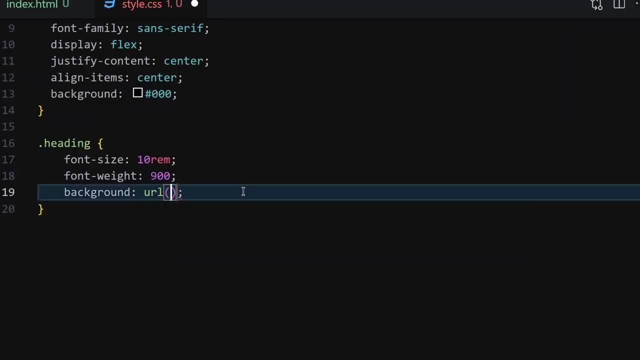 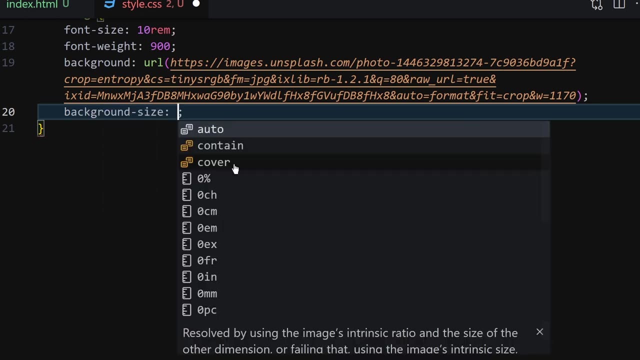 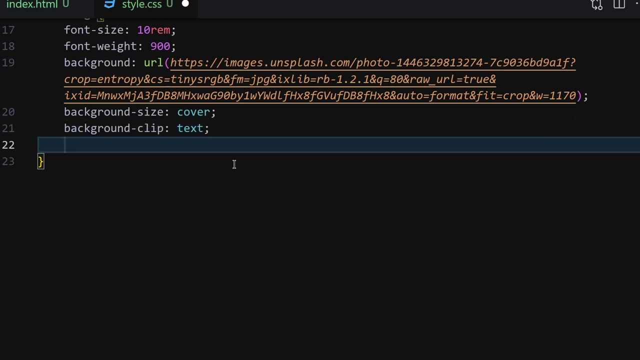 address and then paste it inside a url, and then paste it right here. and what else do we have to do? we have to just provide a background uh size, of color, and then we have to just write a background clip of text, because we want them to be a text, and then we have a webcam background uh clip and we 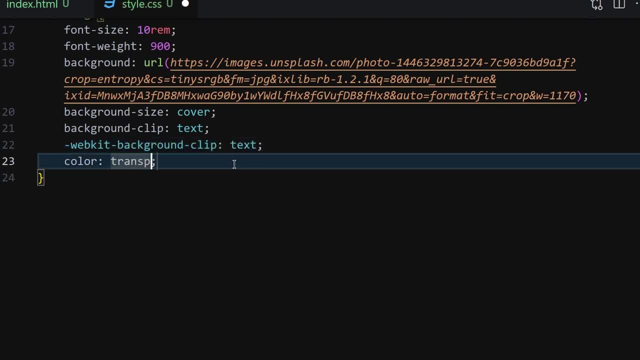 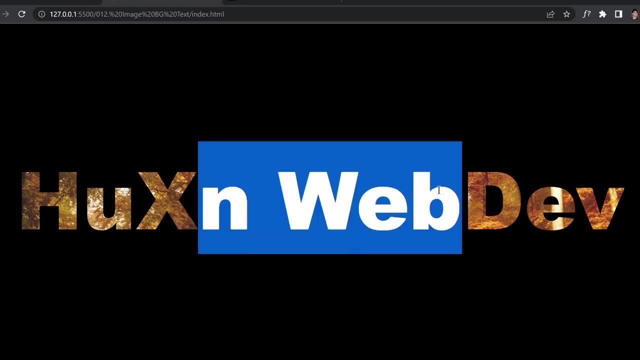 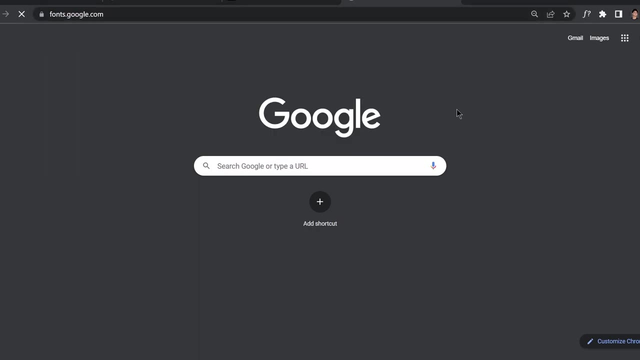 want them to be text as well, and color will be just transparent and cell file, and this is what we get. this is our background image right here, and you can also change the font if you want to. so let's go to fontsgooglecom really quickly. so let me delete my old one. 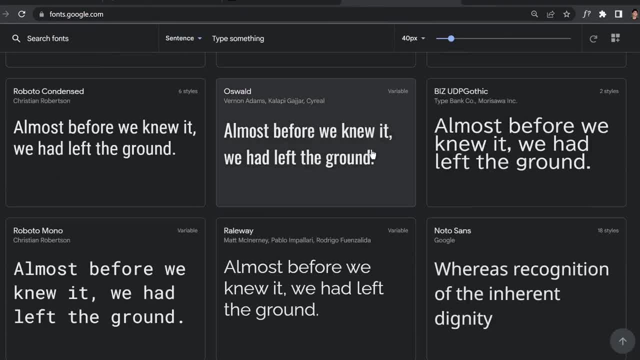 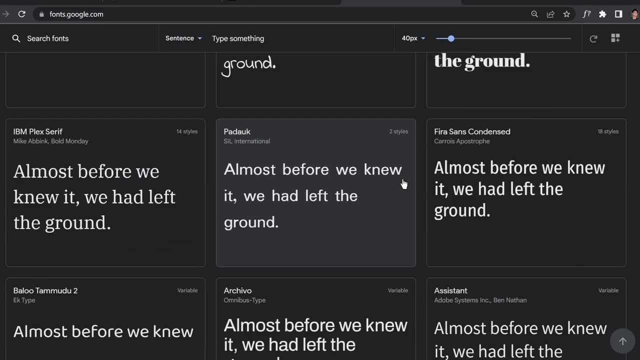 square it out and i don't know which kind of font would be fine for this project. all right, almost before, that's not since, serif, that's not serif, to be precise. you already get the idea, but let me just choose. okay, this one we're going to. 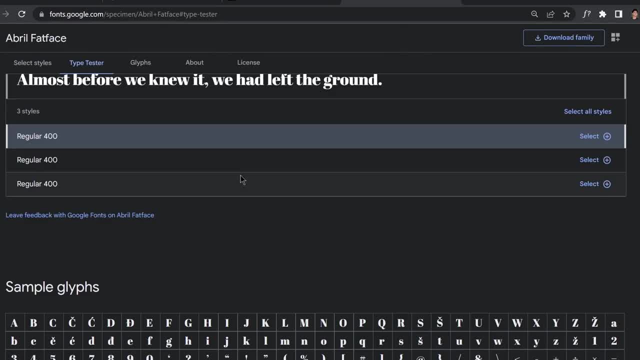 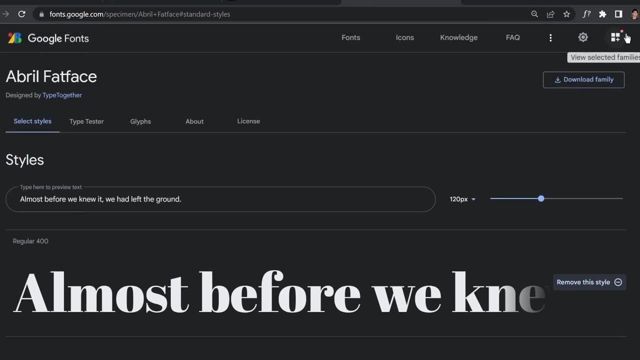 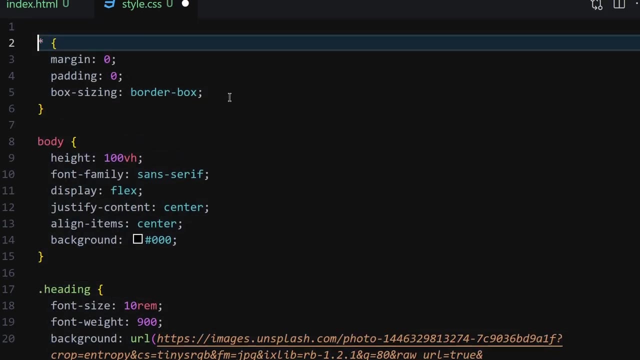 be fine. so yeah, it has just one face. so shout out to this person about the front. just let me grab it um, click on it and this is the font family. so now let's import it in a top of the file and what will be the font family? so now let's import it in a top of the file and what will be? the font family? so now let's import it in a top of the file and what will be?